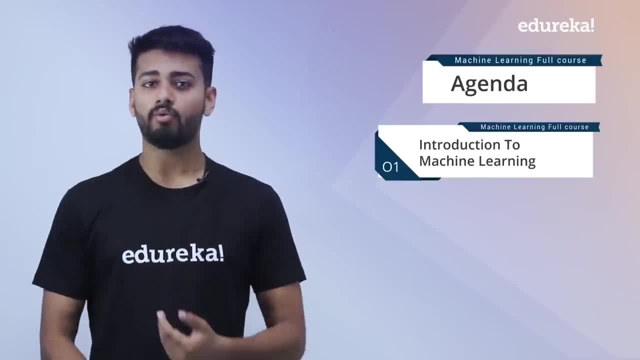 We'll start our first module with introduction to machine learning. Here we'll discuss things like what exactly is machine learning, how it differs from artificial intelligence and deep learning, what are its various types, what are its various applications and finally we'll end our first. 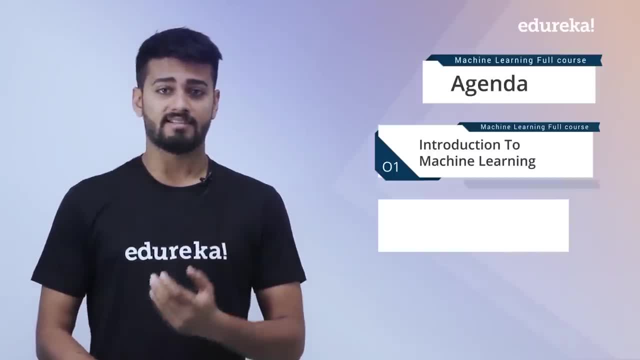 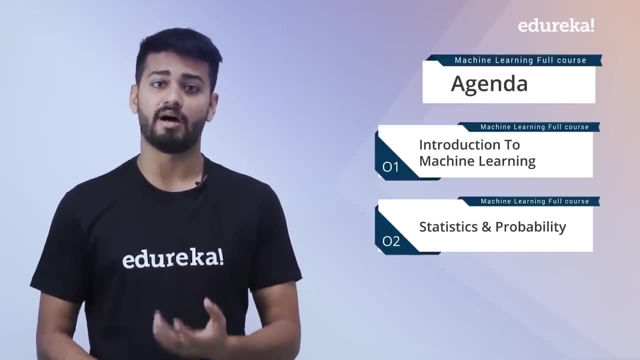 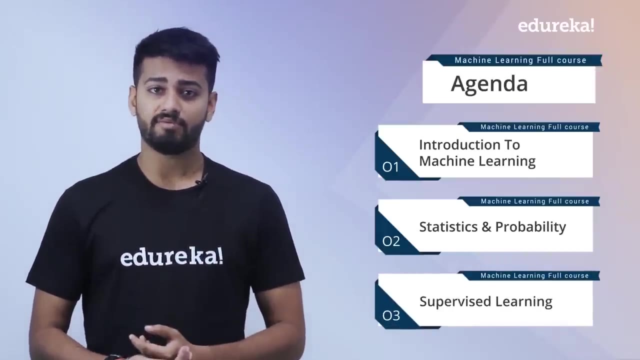 module with a basic demo in Python. Okay, our second module focuses on stats and probability. Here we'll cover things like descriptive statistics, inferential statistics, probability theory and so on. Our third module is on supervised learning. Well, supervised learning is one of a type. 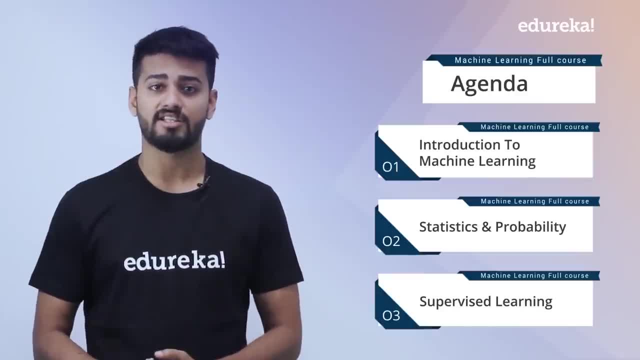 of machine learning which focuses mainly on regression and classification type of problem. It deals with label datasets and the algorithm which are a part of it are linear regression, logistic regression, napias, random forest decision tree and so on. Our fourth module is on unsupervised learning. Well, this is basically a machine learning course, So the last module is on unsupervised learning. Well, this is our first module and we'll end our first module here. So now, before we start, let's discuss a bit about the software. 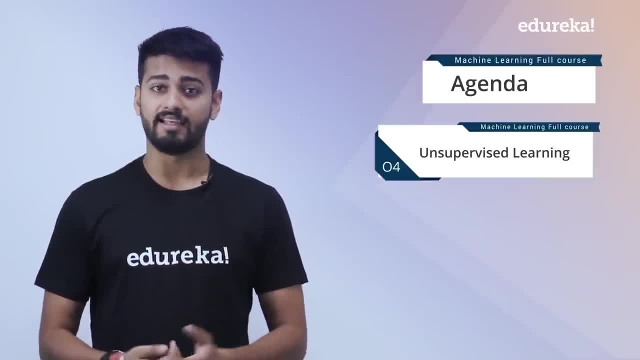 module focuses mainly on dealing with unlabeled data sets, and the algorithm which are a part of it are k-means algorithm and a priori algorithm. as a part of fifth module, we have reinforcement learning. here we are going to discuss about reinforcement learning in depth and also about 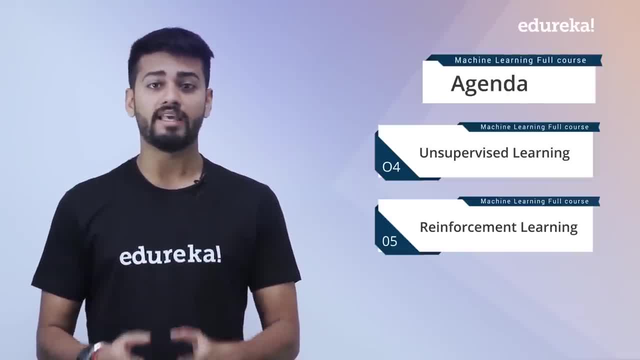 q learning algorithm. finally, in the end, it's all about to make you industry ready. okay, so here we are going to discuss about three different projects which are based on supervised learning, unsupervised learning and reinforcement learning. finally, in the end, i'll tell you about some of the 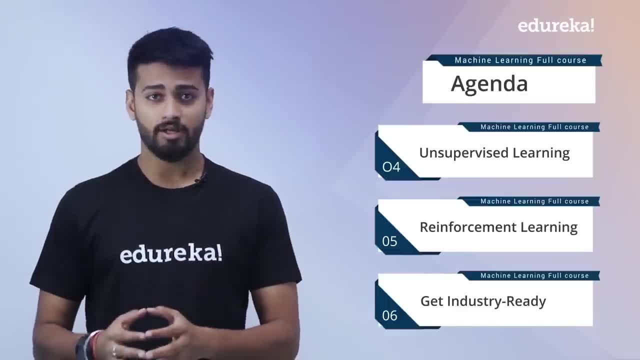 skills that you need to become a machine learning engineer. okay, and also i'll be discussing about some of the important questions that are asked in a machine learning interview. fine, with this, we come to the end of this agenda. before you move ahead, don't forget to subscribe to edureka. 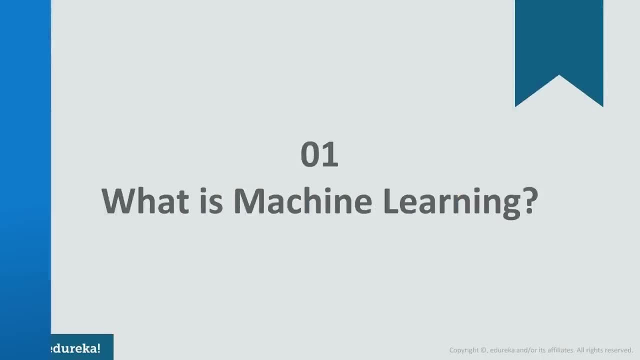 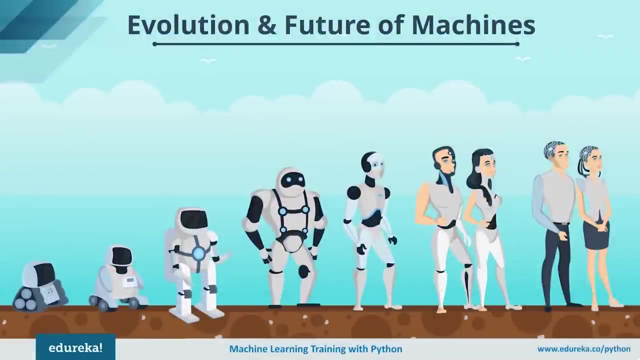 and press the bell icon to never miss any update from us. hello everyone. this is atul from edureka, and welcome to today's session on what is machine learning. as you know, we are living in a world of humans and machines. humans have been evolving and learning from the 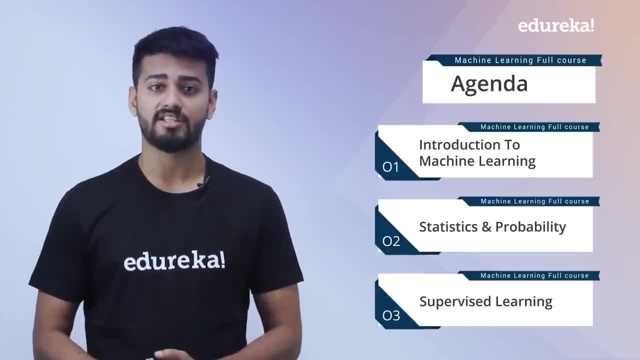 of machine learning which focuses mainly on regression and classification type of problem. It deals with labeled data sets and the algorithms which are a part of it are linear regression, logistic regression, NaPyS, random forest decision tree and so on. Our fourth module, 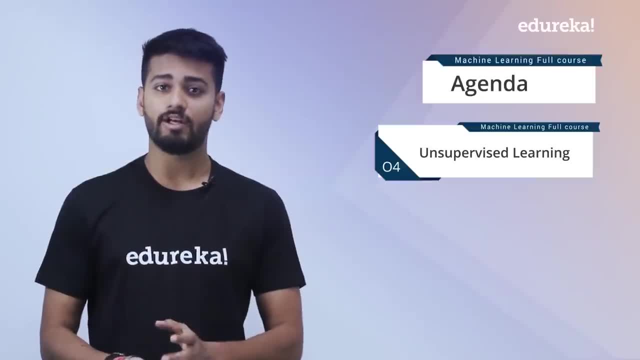 is on unsupervised learning. Well, this module focuses mainly on dealing with unlabeled datasets, and the algorithms which are a part of it are K-Means Algorithm and Apriori Algorithm. As a part of 5th module, we have reinforcement learning. here we are going to discuss about 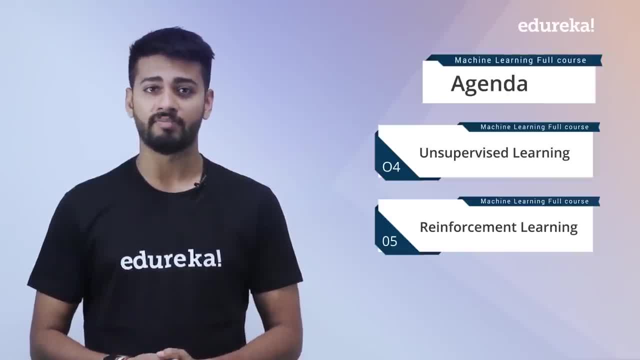 reinforcement, learning in depth, and also about Q-Learning Algorithm. Finally, in the end, it's all about to make you industry ready. okay, so here we are going to discuss about 3 different projects which are based on supervised learning- unsupervised. 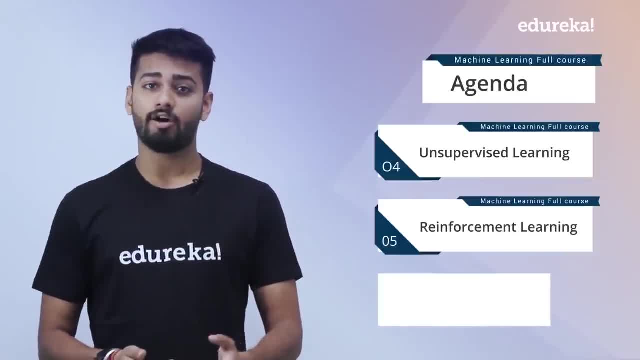 learning and reinforcement learning. Finally, in the end, I will tell you about some of the skills that you need to become a machine learning engineer. okay, and also I will be discussing about some of the important questions that are asked in a machine learning interview. fine, with this, we come to the 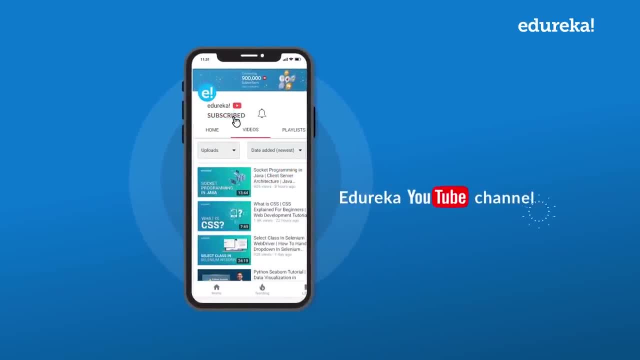 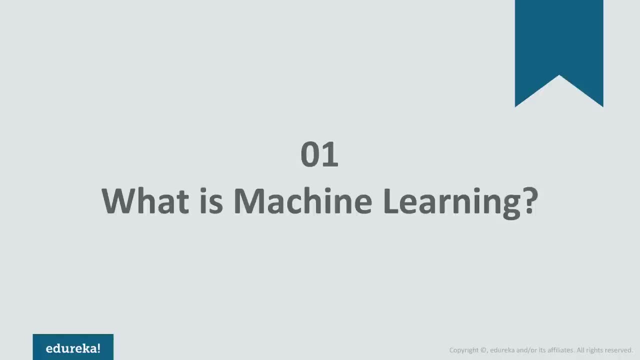 end of this agenda. before you move ahead, don't forget to subscribe to Edureka and press the bell icon to never miss any update from us. Hello everyone, This is Atul from Edureka and welcome to today's session on what is machine learning. 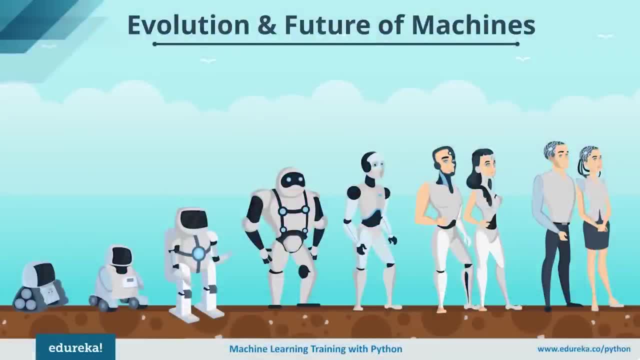 As you know, we are living in a world of humans and machines. humans have been evolving and learning from the past experience since millions of years. On the other hand, the era of machines and robots have just begun. in today's world, These machines or the robots are like. they need to be programmed before they actually. 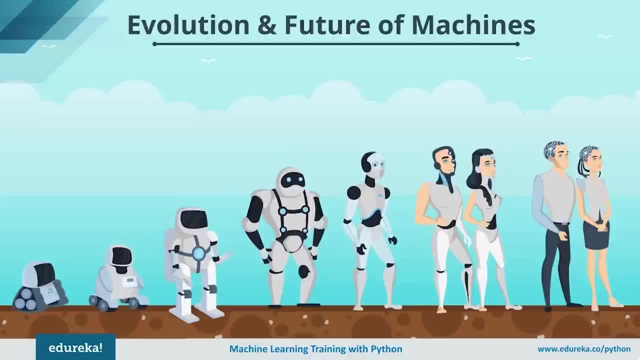 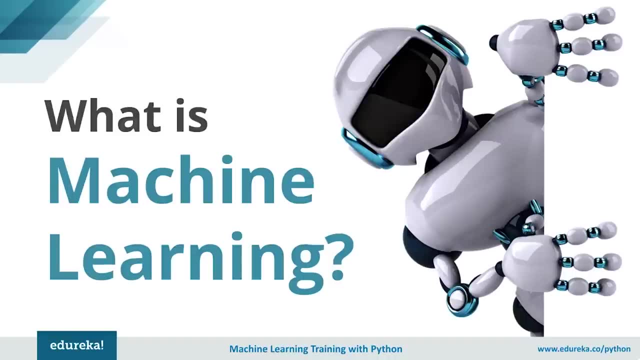 follow your instructions, But what if the machine started to learn on their own? and this is where machine learning comes into picture. Machine learning is the core of many futuristic technological advancement in our world today, You can see various examples or implementation of machine learning around us, such as Tesla's. 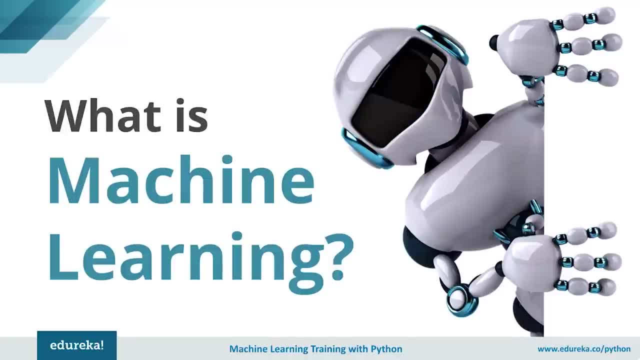 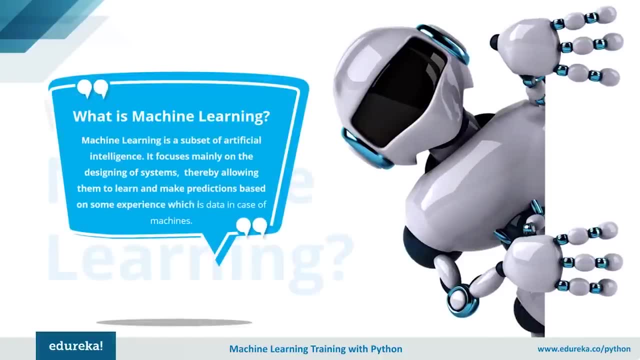 self-driving car, Apple, Siri, Sofia, AI, robot and many more are there. So what exactly is machine learning? Well, machine learning is a subfield of artificial intelligence that focuses on the design of system that can learn from and make decisions and predictions based on the experience, which 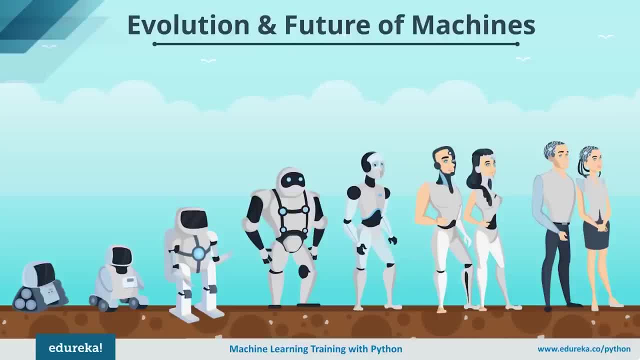 past experience since millions of years. on the other hand, the era of machines and robots have just begun. in today's world, these machines or the robots are like. they need to be programmed before they actually follow your instructions. but what if the machine started to learn on their own? 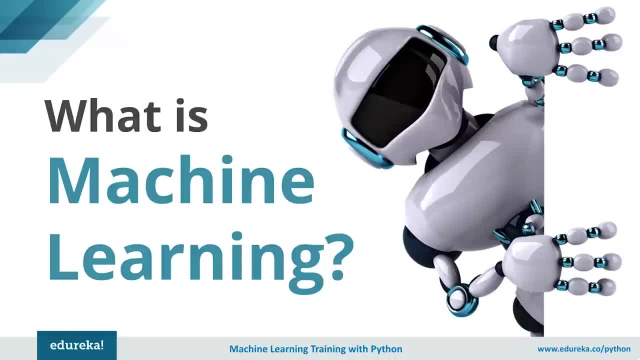 and this is where machine learning comes into picture. machine learning is the core of many futuristic technological advancement in our world. today, you can see various examples or implementation of machine learning around us, such as tesla's self driving car, apple, siri, sofia, ai robot, and many more are there. so what exactly is machine learning? 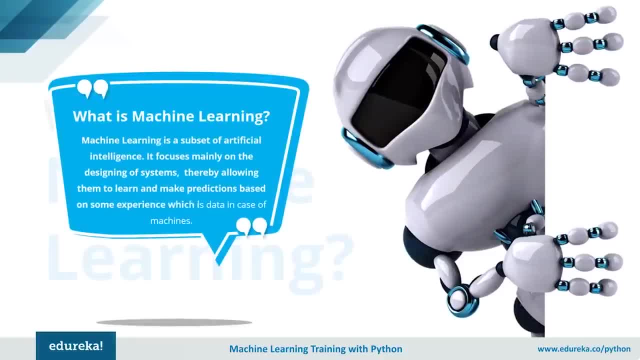 well, machine learning is a subfield of artificial intelligence that focuses on the design of system that can learn from and make decisions and predictions based on the experience, which is data in the case of machine learning machines. machine learning enables computer to act and make data-driven decisions rather. 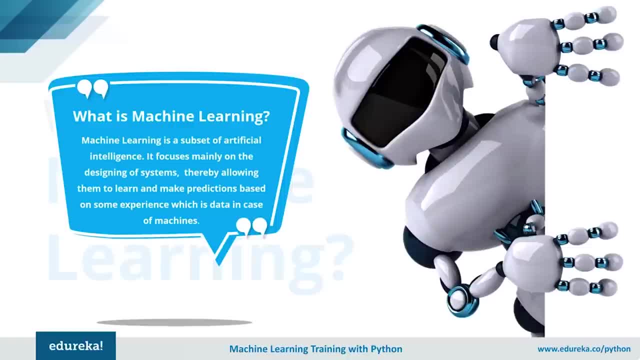 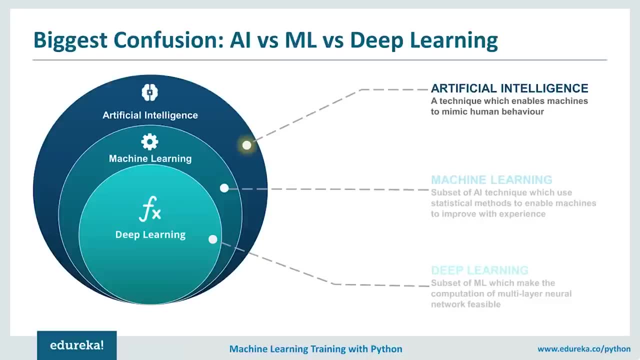 than being explicitly programmed to carry out a certain task, These programs are designed to learn and improve over time when exposed to new data. let's move on and discuss one of the biggest confusion of the people in the world. They think that all the three of them- the AI, the machine learning, 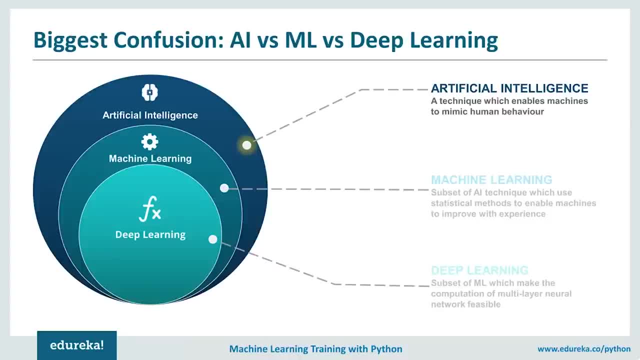 and the deep learning. all the same, You know what they are wrong. Let me clarify things for you. Artificial intelligence is a broader concept of machines being able to carry out task in a smarter way. It covers anything which enables the computer to behave like humans. think of a famous Turing test. 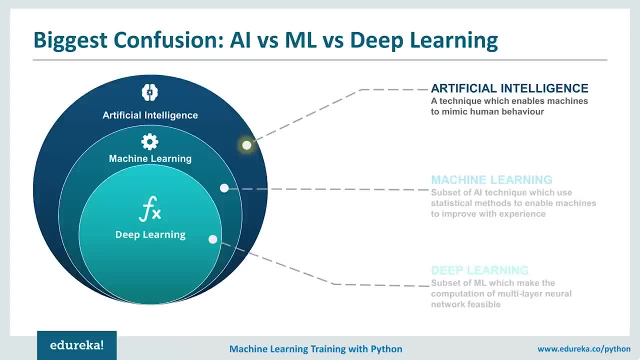 to determine whether a computer is capable of thinking like a human being or not. If you are talking to Siri on your phone and you get an answer, you're already very close to it. So this was about the artificial intelligence. now coming to the machine learning part. 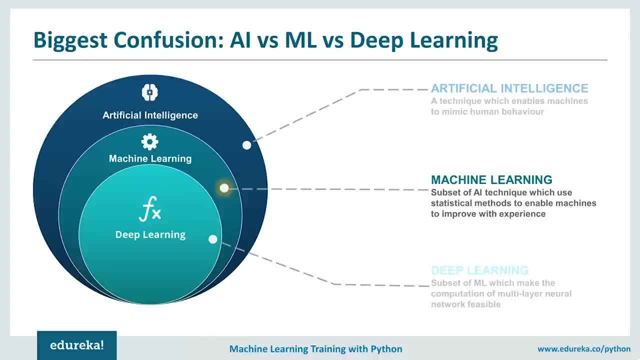 So, as I already said, machine learning is a subset or a current application of AI. It is based on the idea that we should be able to give machine the access to data and let them learn from themselves. It's a subset of artificial intelligence that deals 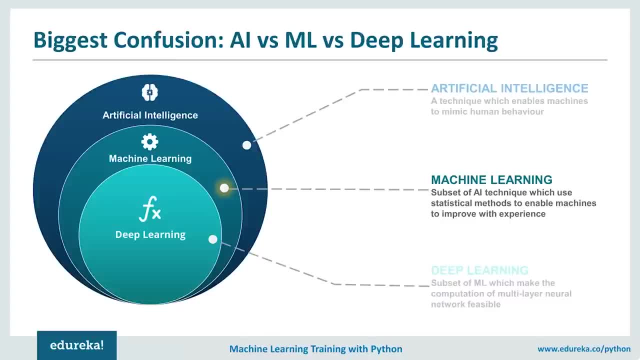 with the extraction of pattern from data set. This means that the machine can not only find the rules for optimal behavior, but also can adapt to the changes in the world. Many of the algorithms involved have been known for decades- centuries, even thanks to the advances. 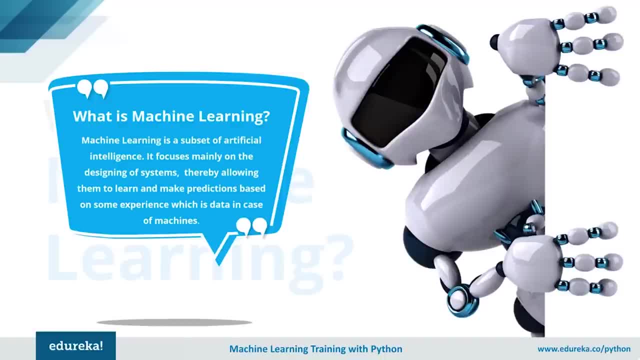 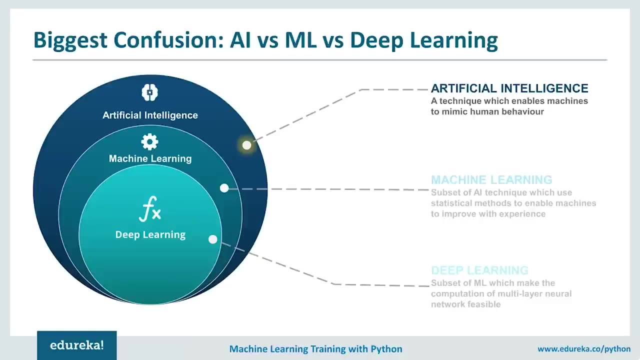 is data in the case of machines, Machine learning enables computer to act and make data-driven decisions. rather than being explicitly programmed to carry out a certain task, These programs are designed to learn and improve over time when exposed to new data. Let's move on and discuss one of the biggest confusion of the people in the world. 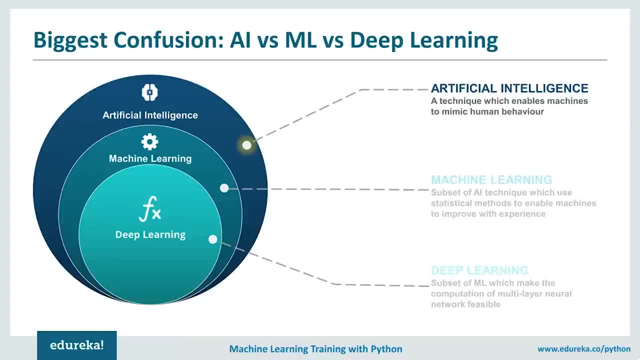 They think that all the three of them- the AI, the machine learning and the deep learning. all the same, You know what they are wrong. Let me clarify things for you. artificial intelligence is a broader concept of machines being able to carry out task in a smarter way. 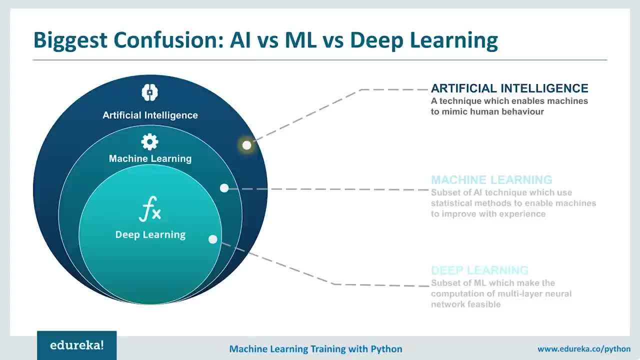 It covers anything which enables the computer to behave like humans. think of a famous Turing test to determine whether a computer is capable of thinking like a human being or not. If you are talking to City on your phone and you get an answer, you're already very close. 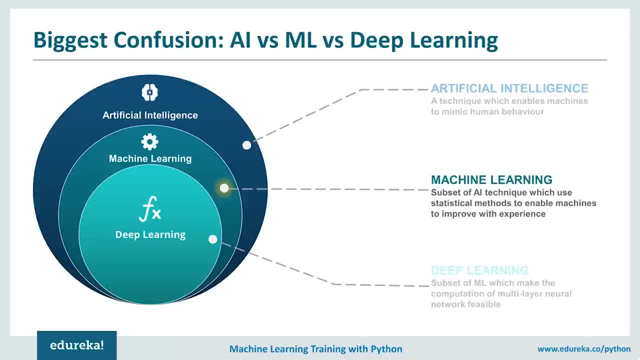 to it. So this was about the artificial intelligence. now coming to the machine learning part. So, as I already said, machine learning is a subset or a current application of AI. It is based on the idea that we should be able to give machine the access. 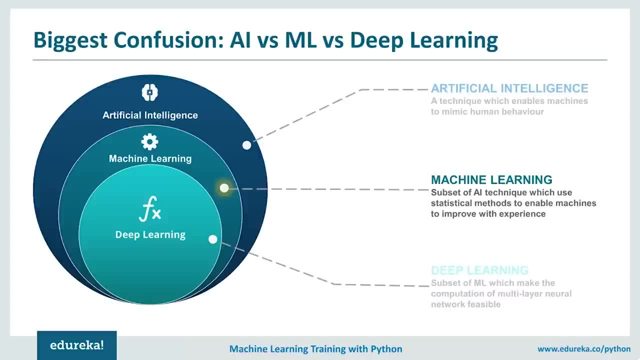 to data and let them learn from themselves. It's a subset of artificial intelligence that deals with the extraction of pattern from data set. This means that the machine can not only find the rules for optimal behavior, but also can adapt to the changes in the world. many of the algorithms involved have been 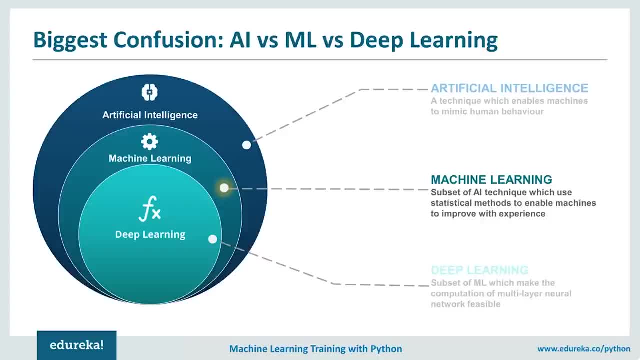 known for decades, centuries. even thanks to the advances in the computer science and panel computing, They can now scale up to massive data volumes. So this was about the machine learning part. now coming over to deep learning. Deep learning is a subset of machine learning where similar machine learning algorithm 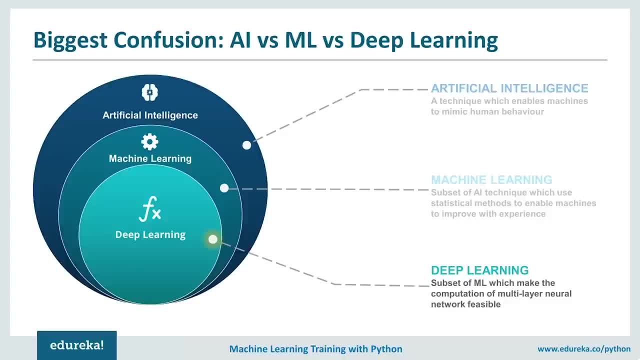 are used to train deep neural network So as to achieve better accuracy in those cases where former was not performing up to the mark. right, I hope now you understood that machine learning, AI and deep learning- all three are different. Okay, moving on ahead. 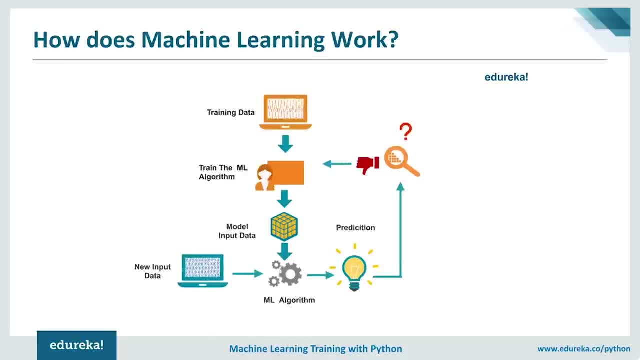 Let's see in general how a machine learning work. One of the approaches is where the machine learning algorithm is trained using a labeled or unlabeled training data set to produce a model. New input data is introduced to the machine learning algorithm and it make prediction based on the model. 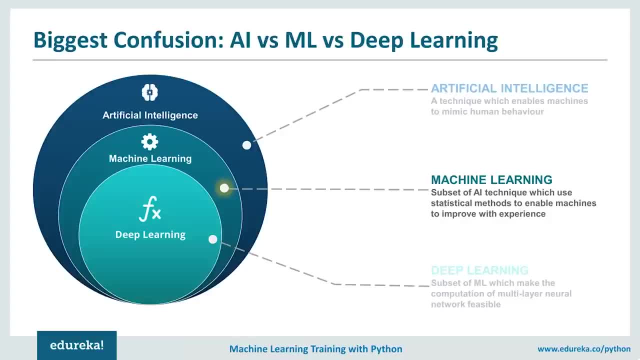 in the computer science and panel computing. They can now scale up to massive data volumes. So this was about the machine learning part. now coming over to deep learning. deep learning is a subset of machine learning where similar machine learning algorithm are used to train deep neural network. 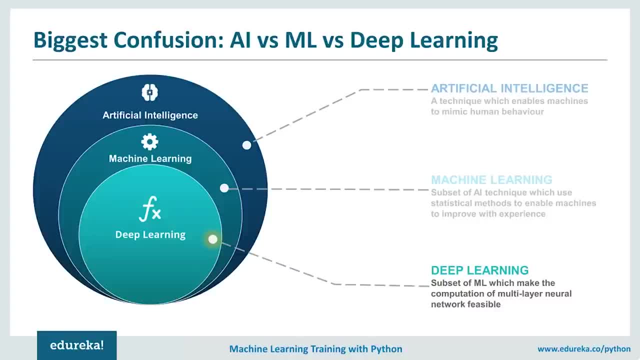 So as to achieve better accuracy in those cases where former was not performing up to the mark. right, I hope now you understood that machine learning, AI and deep learning- all three are different. Okay, moving on ahead, Let's see in general how a machine learning work. 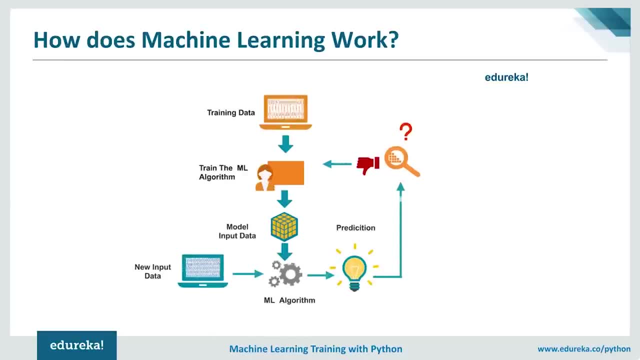 One of the approaches is where the machine learning algorithm is trained using a label or unlabeled training data set to produce a model. new input data is introduced to the machine learning algorithm and it make prediction based on the model. The prediction is evaluated for accuracy and if the accuracy is acceptable. 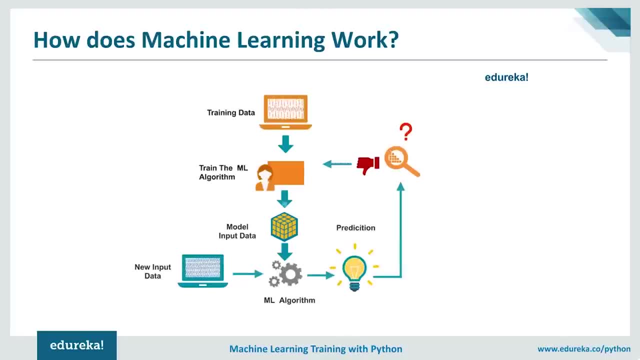 the machine learning algorithm is deployed. Now if the accuracy is not acceptable, the machine learning algorithm is trained again and again with an augmented training data set. This was just in high-level example, as there are many more factor and other steps involved in it. 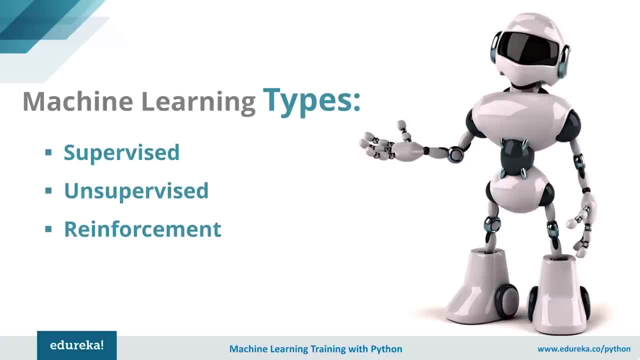 Now let's move on and subcategorize the machine learning into three different types: The supervised learning, unsupervised learning and reinforcement learning- and let's see what each of them are, how they work and how each of them is used in the field of banking, healthcare. 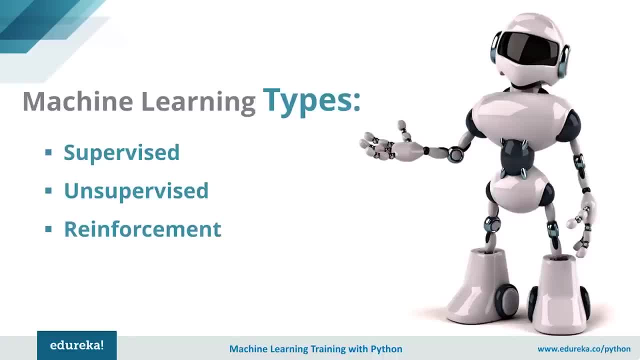 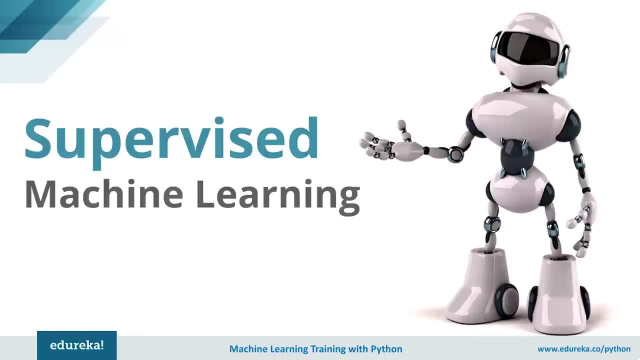 retail and other domains. Don't worry, I'll make sure that I use enough examples and implementation of all three of them to give you a proper understanding of it. So, starting with supervised learning, what is it? So let's see a mathematical definition of supervised learning. 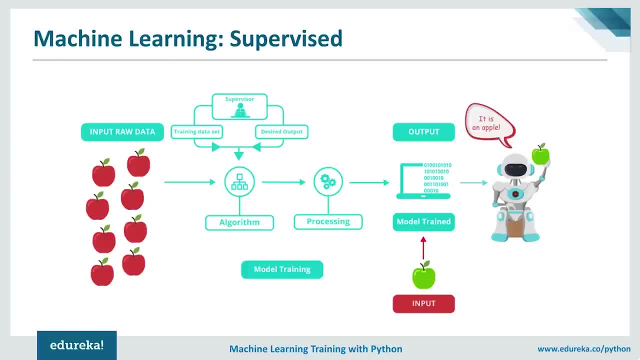 supervised learning is where you have input variables X and an output variable Y and you use an algorithm to learn the mapping function from the input to the output. that is y equal FX. The goal is to approximate the mapping function So well that whenever you have a new input data X. 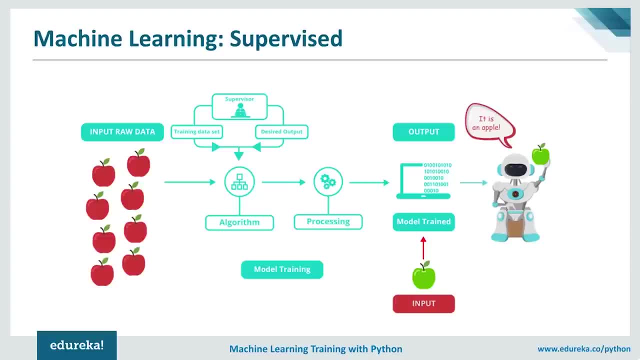 you could predict the output variable, that is Y for that data, Right? I think this was confusing for you. Let me simplify the definition of supervised learning so we can rephrase the understanding of the mathematical definition as a machine learning method where each instances of a training data set. 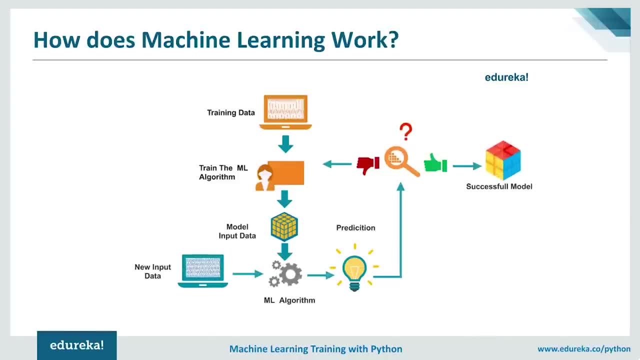 The prediction is evaluated for accuracy and if the accuracy is acceptable, the machine learning algorithm is deployed. Now, if the accuracy is not acceptable, the machine learning algorithm is trained again and again with an augmented training data set. This was just in high-level example, as there are many more factor and other steps involved in it. 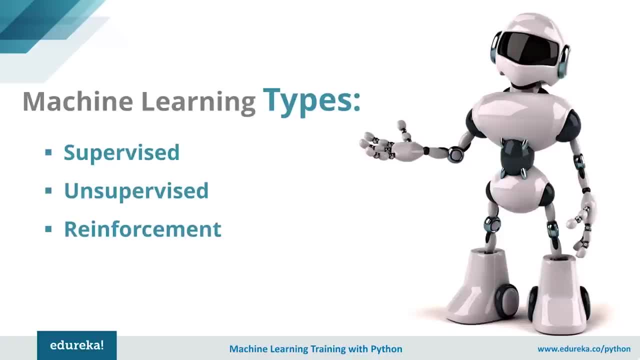 Now let's move on and subcategorize the machine learning into three different types- the supervised learning and supervised learning and reinforcement learning- and let's see what each of them are, how they work and how each of them is used in the field of banking, healthcare, retail. 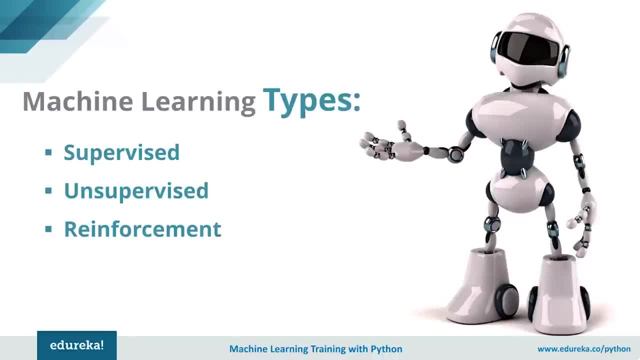 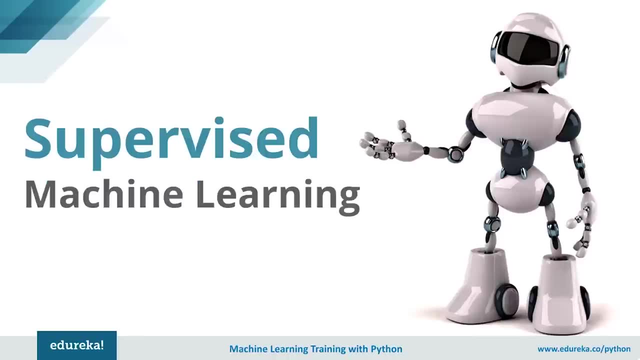 and other domains. Don't worry, I'll make sure that I use enough examples and implementation of all three of them to give you a proper understanding of it. So, starting with supervised learning, what is it? So let's see a mathematical definition of supervised learning. supervised learning. 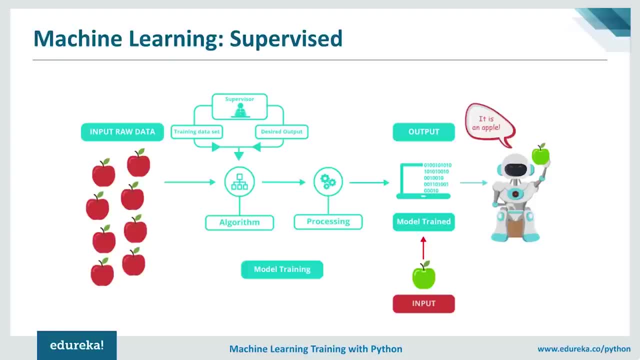 is where you have input variables X and an output variable Y and you use an algorithm to learn the mapping function from the input to the output. that is y equal FX. The goal is to approximate the mapping function So well that whenever you have a new input data X. 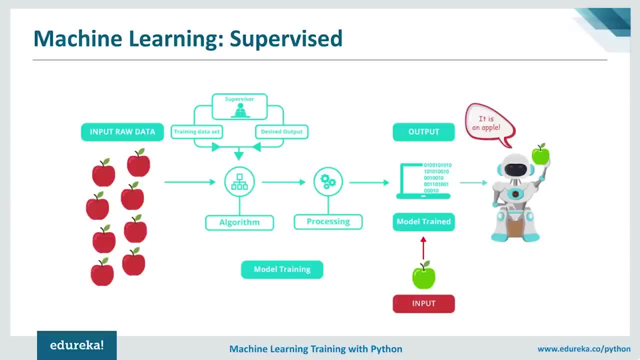 you could predict the output variable, that is Y for that data, right? I think this was confusing for you. Let me simplify the definition of supervised learning so we can rephrase the understanding of the mathematical definition as a machine learning method where each instances of a training data set is composed. 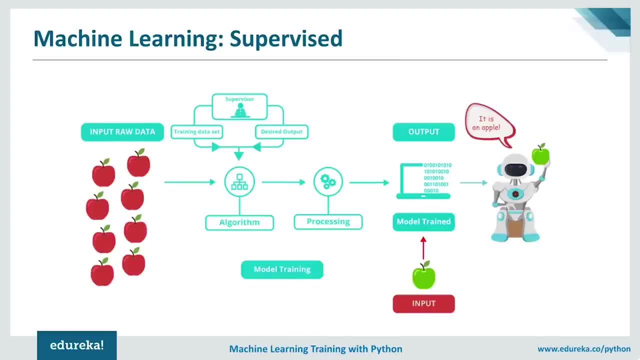 of different input attribute and an expected output. the input attributes of a training data set can be of any kind of data. It can be a pixel of image, It can be a value of a database row, or it can even be a audio frequency histogram. 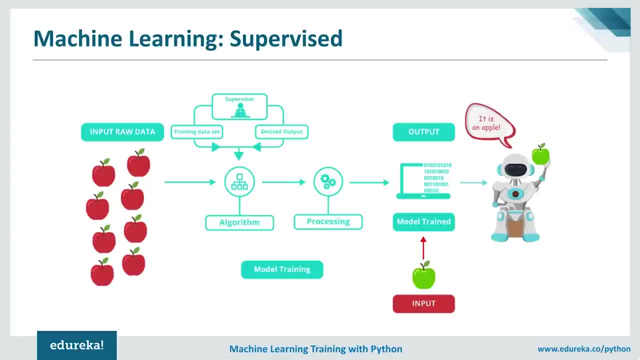 right for each input instance and expected output values associated. The value can be discrete, representing a category, or can be a real or continuous value. in either case, The algorithm learns the input pattern that generate the expected output. Now, once the algorithm is trained, it can be used to predict the correct output of a never seen input. 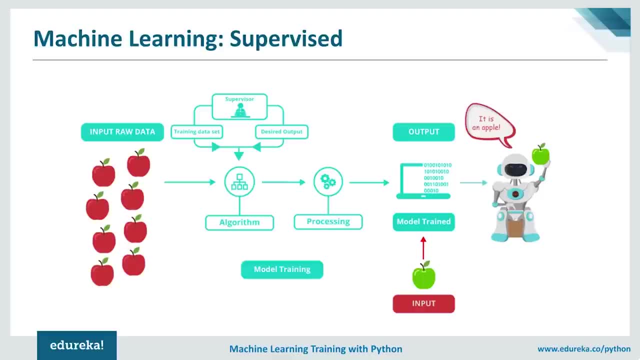 You can see a image on your screen right. in this image You can see that we are feeding raw inputs, as image of Apple, to the algorithm. as a part of the algorithm, We have a supervisor who keeps on correcting the machine or who keeps on training the machine. 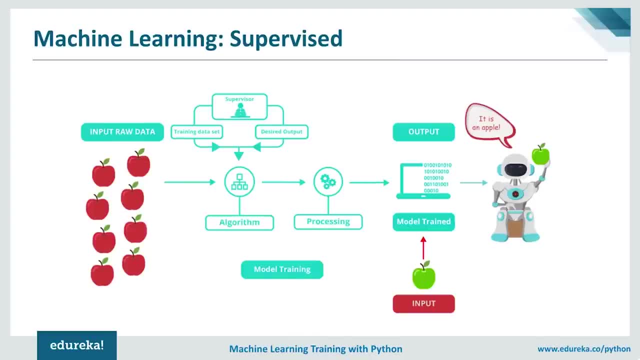 is composed of different input attribute and an expected output. the input attributes of a training data set can be of any kind of data: It can be a pixel of image, It can be a value of a database row, or it can even be a audio frequency histogram right. 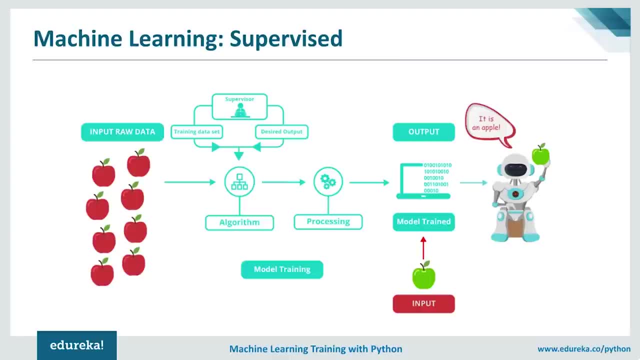 But each input instance and expected output values associated. the value can be discrete, representing a category, or can be a real or continuous value. in either case, The algorithm learns the input pattern that generate the expected output. Now, once the algorithm is trained, it can be used to predict the correct output. 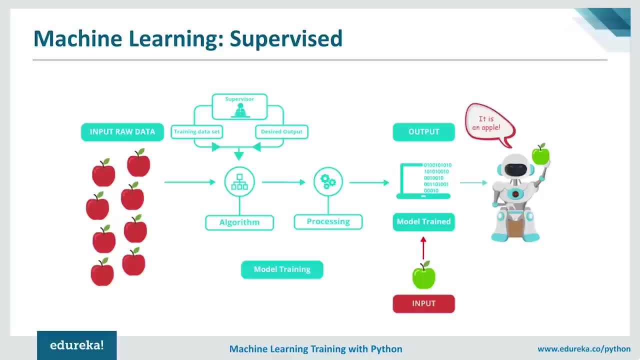 of a never seen input. You can see a image on your screen right. in this image You can see that we are feeding raw inputs as image of Apple to the algorithm. as a part of the algorithm, We have a supervisor who keeps on correcting the machine. 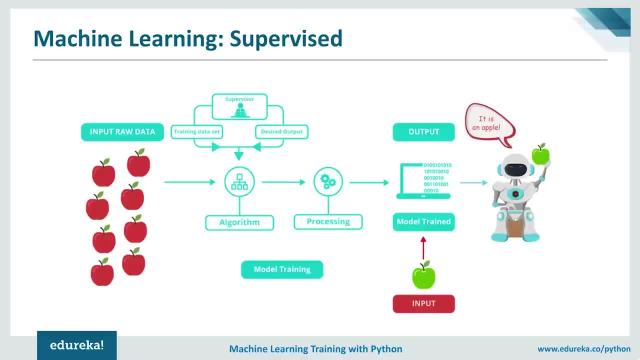 or who keeps on training the machine. It keeps on telling him that, yes, it is an apple, No, it is not an apple, things like that. So this process keeps on repeating until we get a final train model, Once the model is ready. 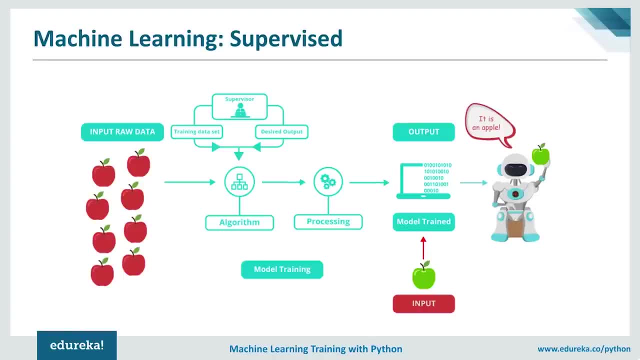 it can easily predict the correct output of a never seen input. in this slide, You can see that we are giving an image of a green apple to the machine and the machine can easily identify it as, yes, it is an apple and it is giving the correct result, right? 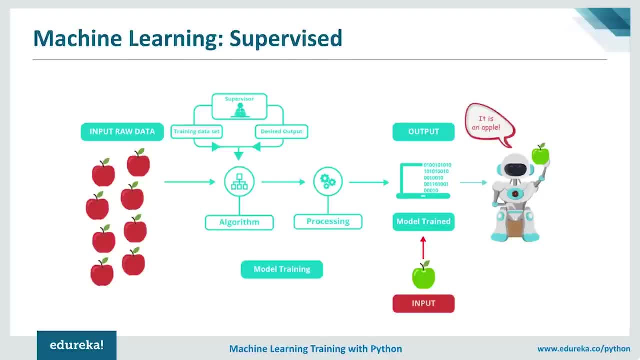 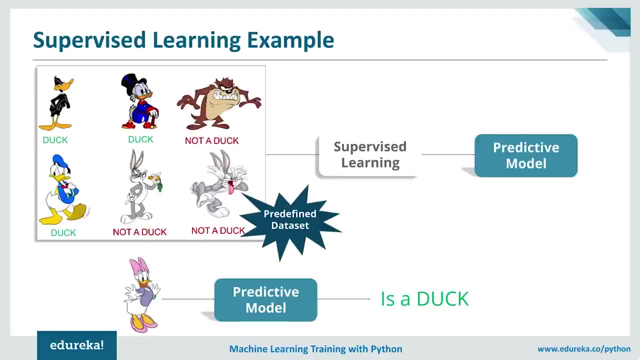 Let me make things more clearer to you, Let's discuss another example of it. So in this slide, the image shows an example of a supervised learning process used to produce a model which is capable of recognizing the ducks in the image. The training data set is composed of labeled picture. 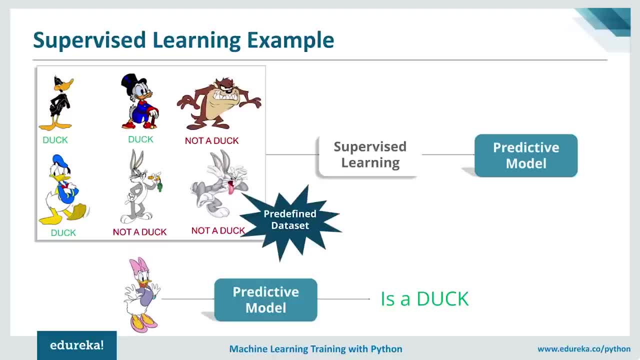 of ducks and non-ducks. the result of supervised learning process is a predictive model which is capable of associating a label- duck or not duck- to the new image presented to the model. Now one strain: the resulting predictive model can be deployed to the production environment. 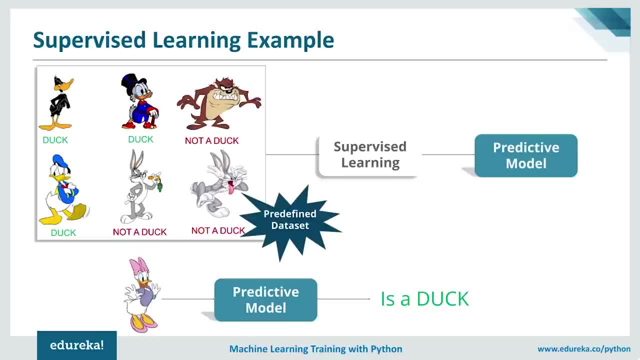 You can see a mobile app, For example. once deployed, it is ready to recognize the new pictures right now. You might be wondering why this category of machine learning is named as supervised learning. Well, it is called as supervised learning because the process of an algorithm learning 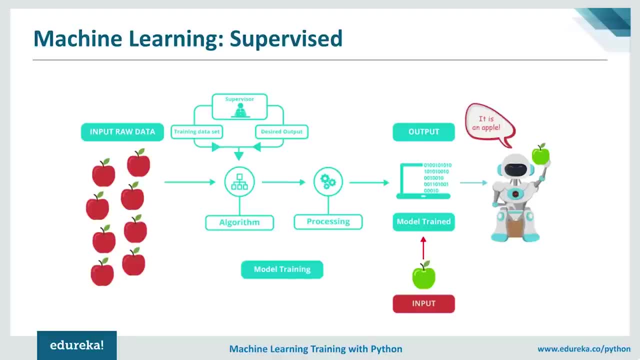 It keeps on telling him that yes, it is an apple and no, it is not an apple, things like that. So this process keeps on repeating until we get a final train model. Once the model is ready, it can easily predict the correct output of a never seen input. 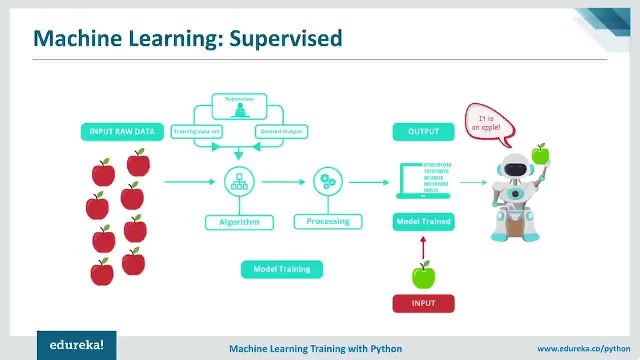 in this slide, You can see that we are giving an image of a green apple to the machine, and the machine can easily identify it as, yes, it is an apple and it is giving the correct result, right? Let me make things more clearer to you. 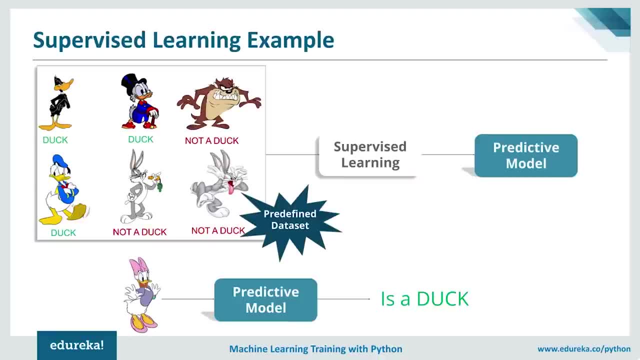 Let's discuss another example of it. So in this slide the image shows an example of a supervised learning process used to produce a model which is capable of recognizing the ducks in the image. The training data set is composed of labeled picture of ducks and non-ducks. 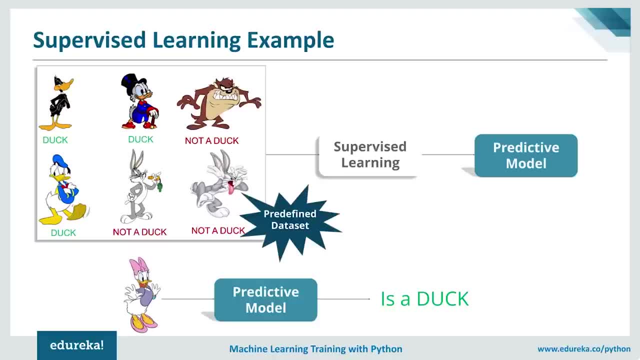 The result of supervised learning process is a predictor model which is capable of associating a label- duck or not duck- to the new image presented to the model. Now one strain: the resulting predictive model can be deployed to the production environment. You can see a mobile app. 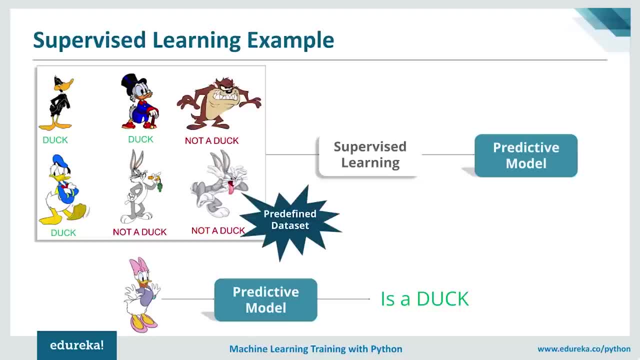 For example, once deployed, it is ready to recognize the new pictures right now. You might be wondering why this category of machine learning is named as supervised learning. Well, it is called as supervised learning because the process of an algorithm learning from the training data set. 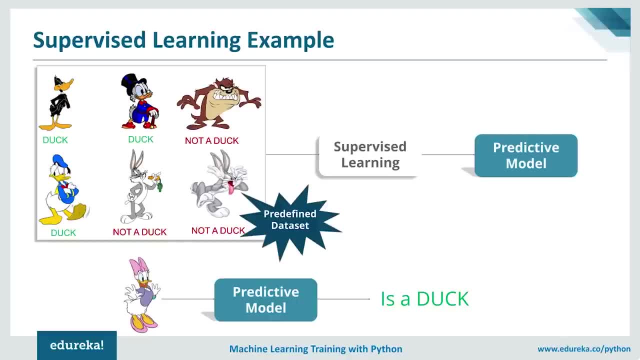 can be thought of as a teacher supervising the learning process. We know the correct answers the algorithm iteratively makes while predicting on the training data and is corrected by the teacher. the learning stops when the algorithm achieves an acceptable level of performance. Now let's move on and see some 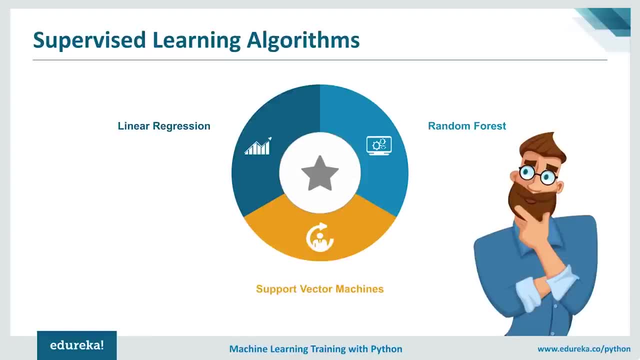 of the popular supervised learning algorithm. So we have linear regression, random Forest and support vector machines. These are just for your information. We'll discuss about these algorithms in our next video. Now let's see some of the popular use cases of supervised learning. 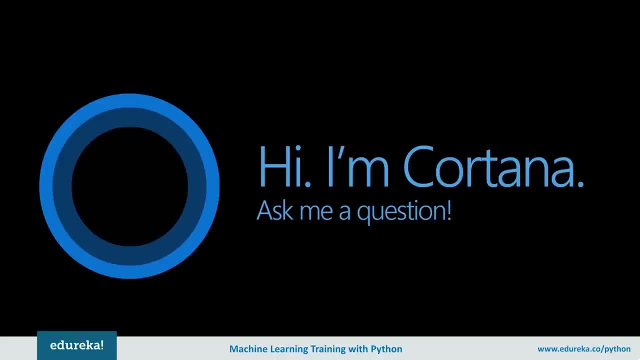 So we have Cortana, Cortana or any other speech automation in your mobile phone trains using your voice and one strain. it start working based on the training. This is an application of supervised learning. suppose you are telling, okay, Google call Sam. or you say, hey, Siri, call Sam, you get an answer. 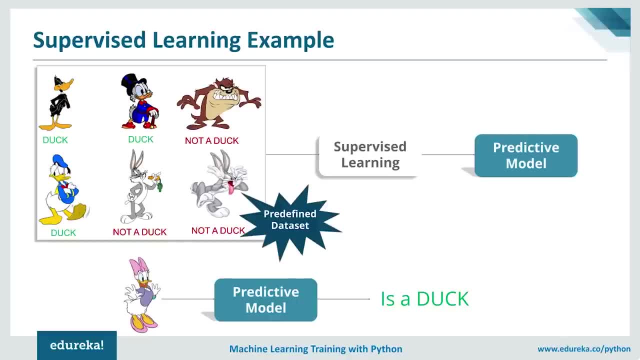 from the training data set can be thought of as a teacher supervising the learning process. We know the correct answers the algorithm iteratively makes while predicting on the training data and is corrected by the teacher. the learning stops when the algorithm achieves an acceptable level of performance. now let's move on and see some. 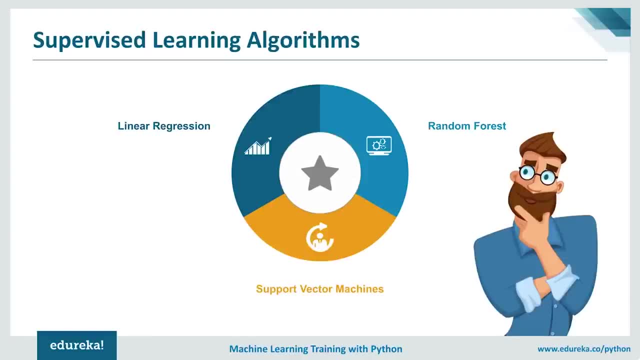 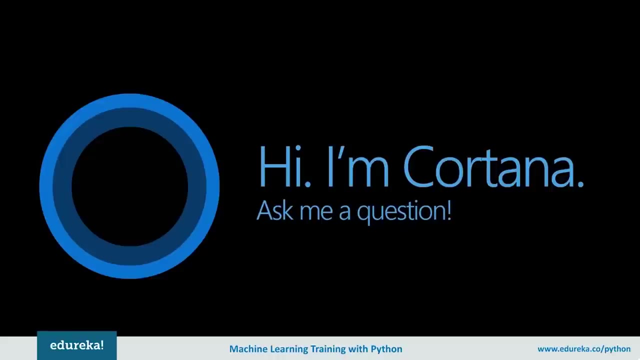 of the popular supervised learning algorithm. So we have linear regression, random Forest and support vector machines. These are just for your information. will discuss about these algorithms in our next video. Now let's see some of the popular use cases of supervised learning. So we have Cortana, Cortana. 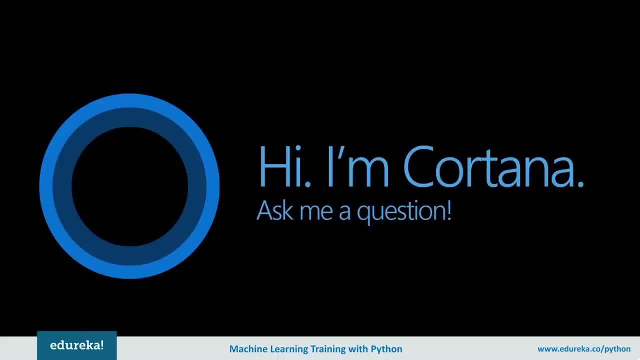 or any other speech automation in your mobile phone trains using your voice and once train it start working based on the training. This is an application of supervised learning. suppose you are telling, okay, Google, call Sam. or you say, hey, Siri, call Sam, you get an answer to it. 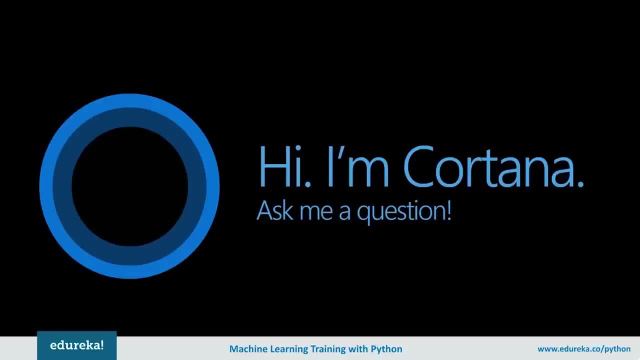 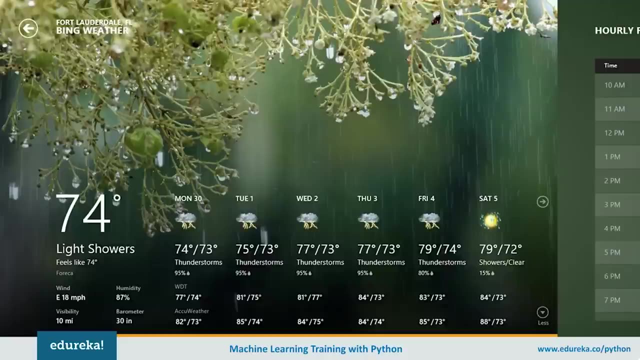 and action is performed and automatically a call goes to Sam. So these are just an example of supervised learning. next comes the weather app based on some of the prior knowledge, like when it is sunny the temperature is higher, when it is cloudy, humidity is higher, any kind of that. 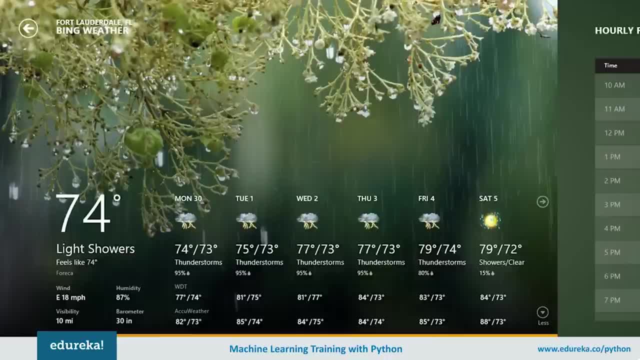 They predict the parameters for a given time. So this is also an example of supervised learning, as you are feeding the data to the machine and telling that whenever it is sunny, the temperature should be higher, whenever it is cloudy, the humidity should be higher. So it's an example of supervised learning. another example: 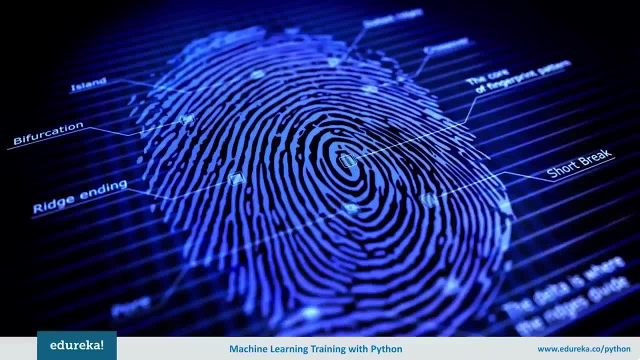 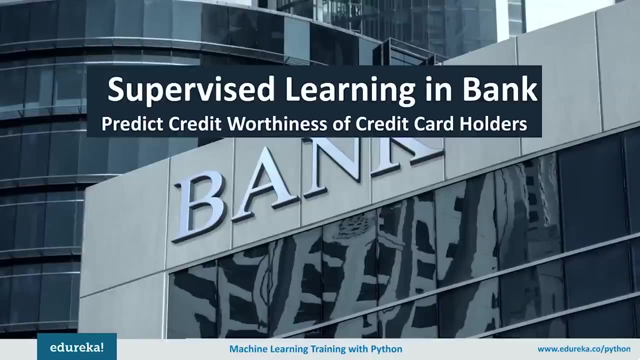 is biometric attendance, Where you train the machine and, after a couple of inputs of your biometric identity, beat your thumb, your iris or your earlobe or anything. once trained, the machine can validate your future input and can identify you. next comes in the field of banking sector. in banking sector supervised. 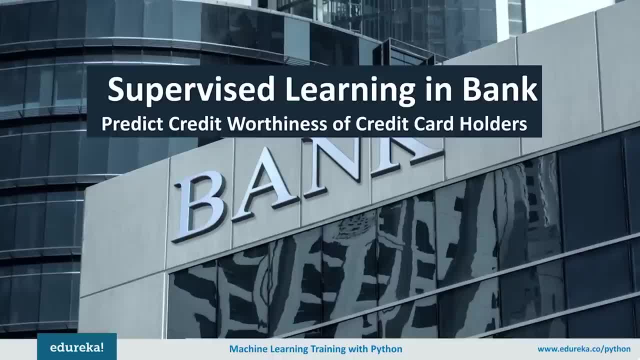 learning is used to predict the credit worthiness of a credit card holder by building a machine learning model to look for faulty attributes, by providing it with a data on delinquent and non delinquent customers. next comes The health care sector. in the health care sector, 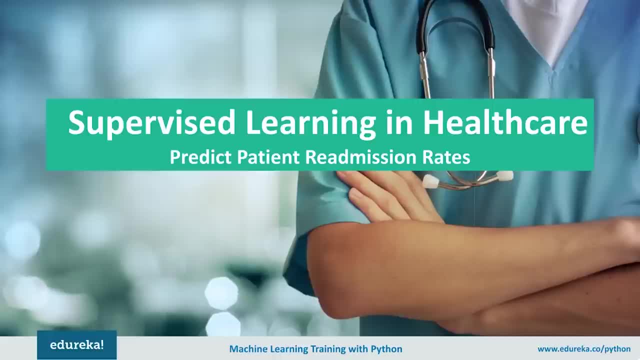 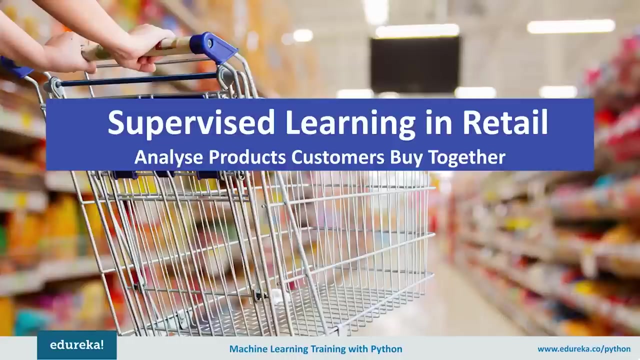 It is used to predict the patient's readmission rates by building a regression model, by providing data on the patient's treatment, administration and readmissions to show variables that best correlate with readmission. next comes the retail sector, and retail sector: It is used to analyze the product. 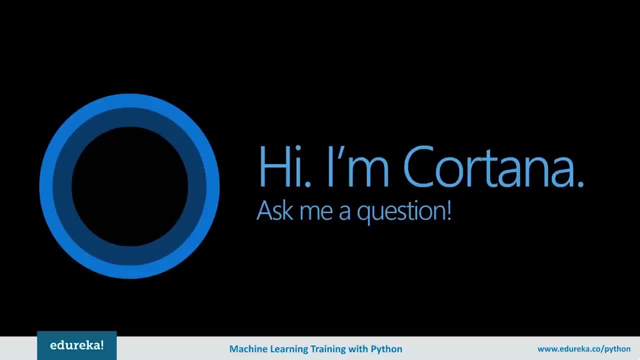 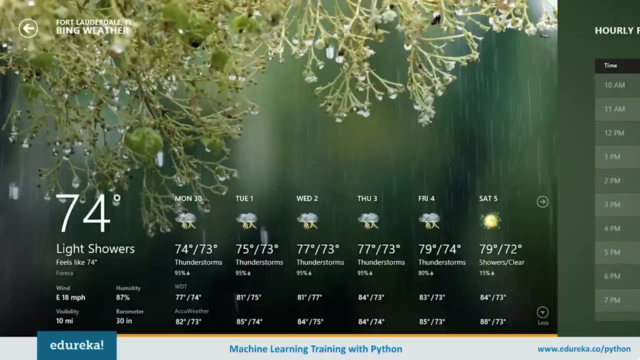 to it and action is performed and automatically a call goes to Sam. So these are just an example of supervised learning. next comes the weather app based on some of the prior knowledge, like when it is sunny the temperature is higher, when it is cloudy, humidity is higher, any kind of that. 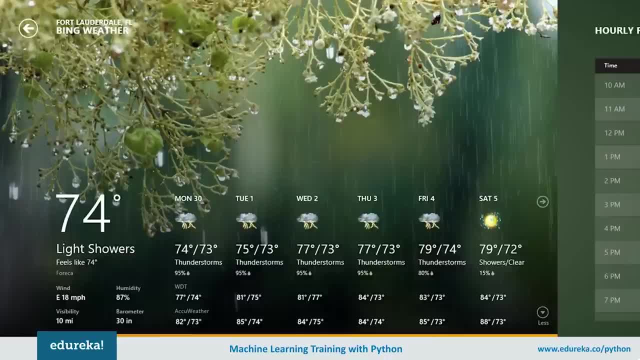 They predict the parameters for a given time. So this is also an example of supervised learning, as you are feeding the data to the machine and telling that whenever it is sunny, the temperature should be higher, whenever it is cloudy, The humidity should be higher. 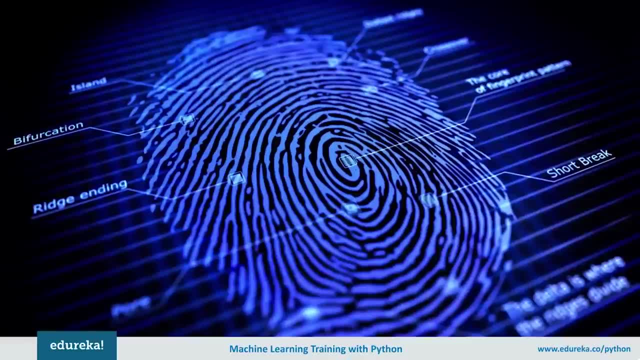 So it's an example of supervised learning. Another example is biometric attendance, Where you train the machine and, after a couple of inputs of your biometric identity, beat your thumb, your iris or your earlobe or anything. once trained, the machine can validate your future input. 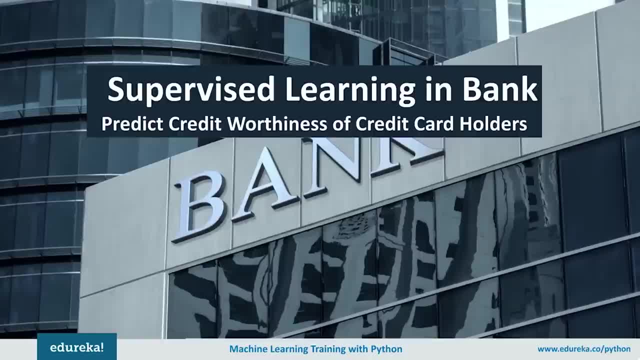 and can identify you. next comes in the field of banking sector. in banking sector, supervised learning is used to predict the credit worthiness of a credit card holder by building a machine learning model to look for faulty attributes, by providing it with a data on delinquent and non delinquent customers. next comes the healthy. 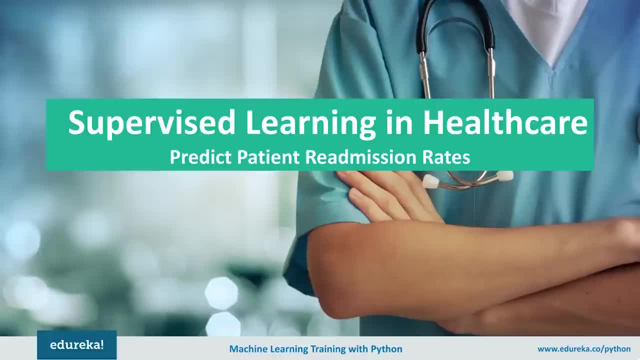 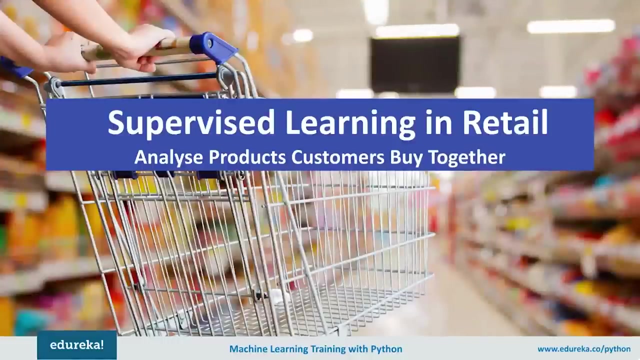 care sector. in the health care sector, It is used to predict the patient's readmission rates by building a regression model, by providing data on the patient's treatment, administration and readmissions to show variables that best correlate with readmission. next comes the retail sector and retail sector. 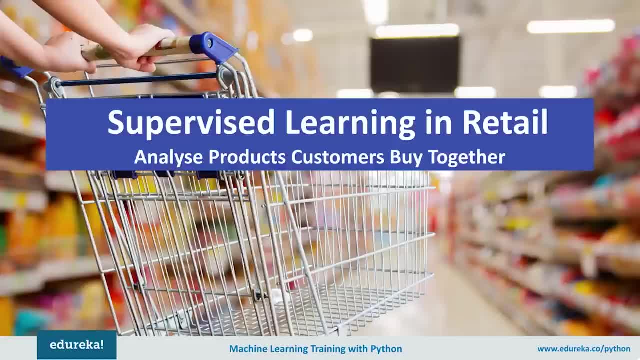 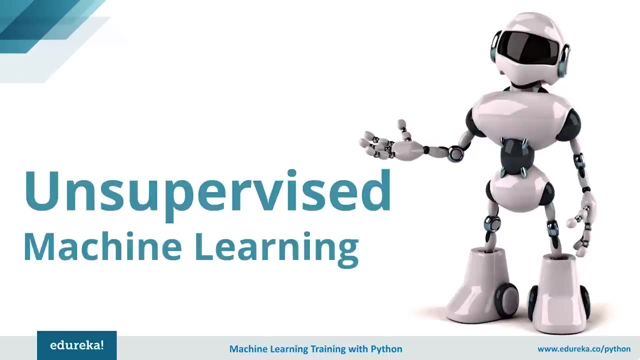 It is used to analyze the product that a customer buy together. It does this by building a supervised model to identify frequent item sets and Association rule from the transactional data. Now let's learn about the next category of machine learning, the unsupervised part, mathematically unsupervised learning. 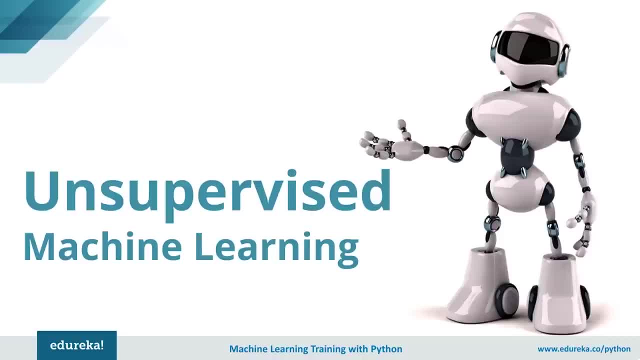 is where you only have input data X and no corresponding output variable. the goal for unsupervised learning is to model the underlining structure or distribution in the data in order to learn more about the data. So let me rephrase you this in simple terms. 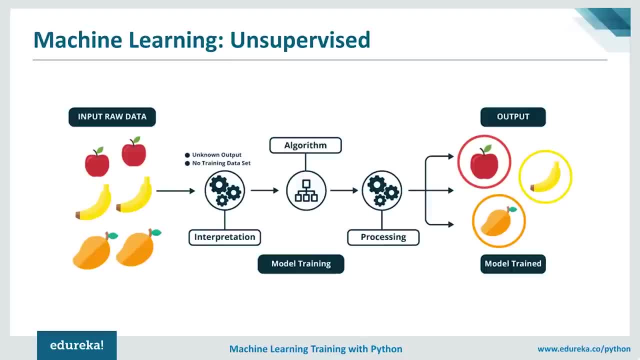 and unsupervised learning approach. the data instances of a training data set do not have an expected output associated to them. instead, unsupervised learning algorithm detects pattern based on in it characteristics of the input data. an example of machine learning task that applies unsupervised learning. 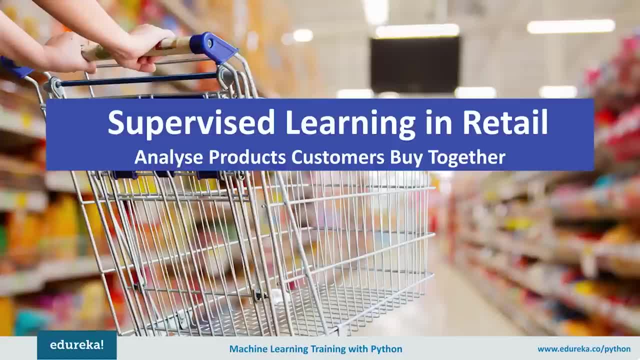 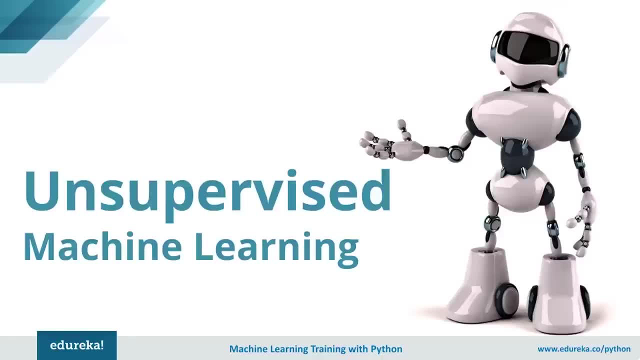 that a customer buy together. It does this by building a supervised model to identify frequent item sets and association rule from the transactional data. Now let's learn about the next category of machine learning, the unsupervised part, mathematically unsupervised learning. 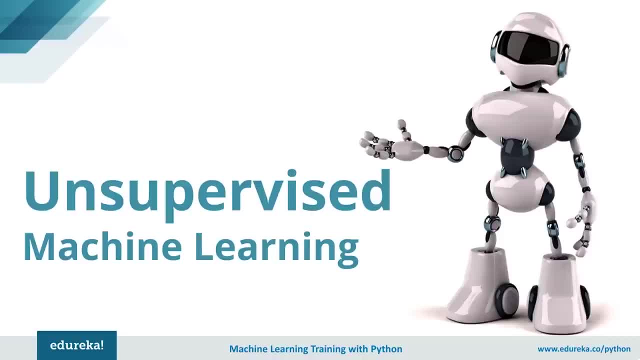 is where you only have input data X and no corresponding output variable. The goal for unsupervised learning is to model the underlining structure or distribution in the data in order to learn more about the data. So let me rephrase you this in simple terms. 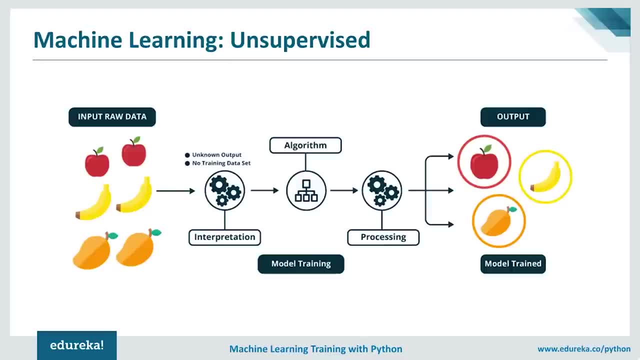 and unsupervised learning approach. the data instances of a training data set do not have an expected output associated to them. instead, unsupervised learning algorithm detects pattern based on in it characteristics of the input data. an example of machine learning task that applies unsupervised learning is clustering. 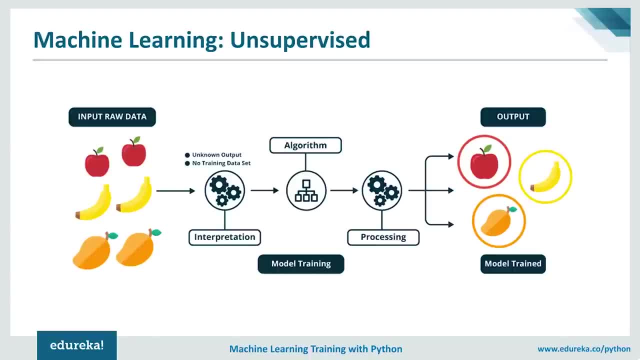 and this task. similar data instances are grouped together in order to identify clusters of data. in this slide You can see that initially we have different varieties of fruits as input. now these set of fruits as input X are given to the model. now was the model is trained. 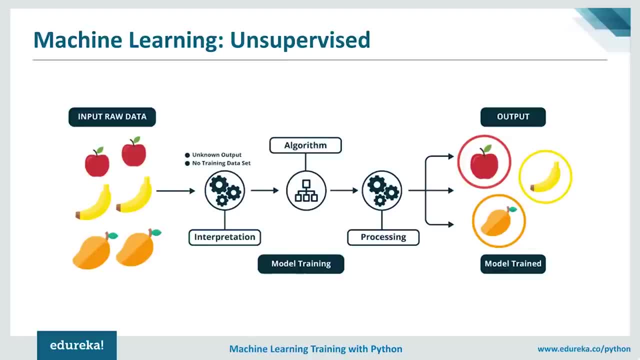 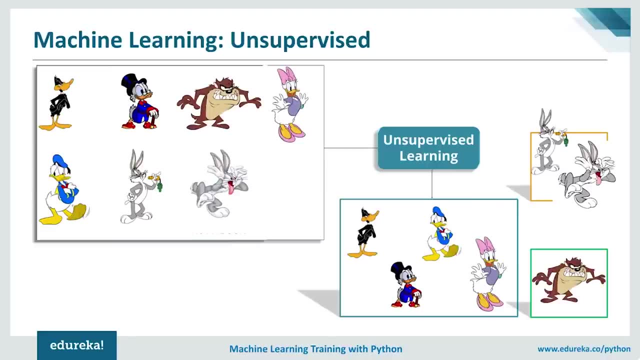 using unsupervised Learning algorithm. The model will create clusters on the basis of its training. It will group the similar fruits and make their cluster. Let me make things more clearer to you. Let's take another example of it. So in this slide, the image below shows an example. 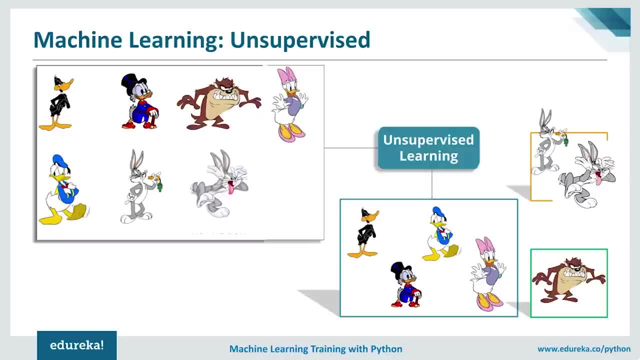 of unsupervised learning process. this algorithm processes an unlabeled training data set and, based on the characteristics, it groups the picture into three different clusters of data. despite the ability of grouping similar data into clusters, The algorithm is not capable to add labels to the group that will guard them only knows. 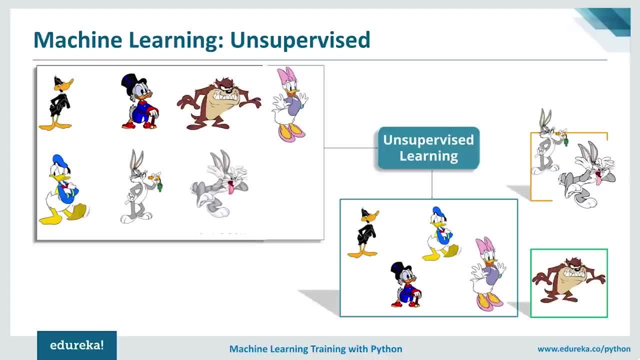 which data instances are similar, but it cannot identify the meaning of this group. So now you might be wondering why this category of machine learning is named as unsupervised learning. So these are called as unsupervised learning because, unlike supervised learning, ever. 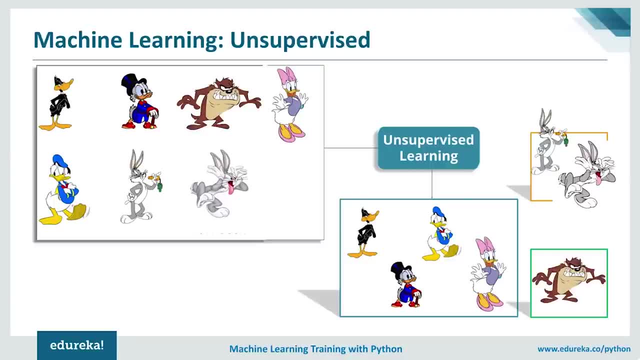 There are no correct answers and there is no teacher. algorithms are left on their own to discover and present the interesting structure in the data. Let's move on and see some of the popular unsupervised Learning algorithm. So we have here K means a Peoria algorithm. 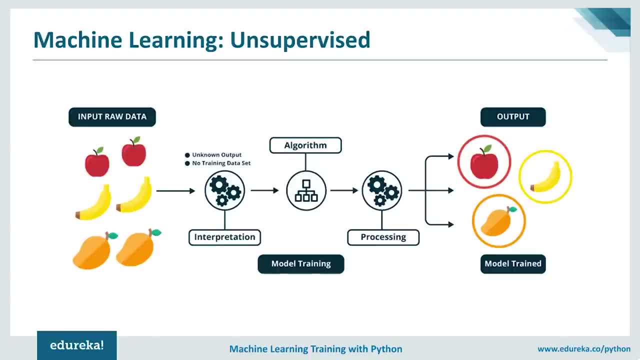 is clustering. in this task, similar data instances are grouped together in order to identify clusters of data. in this slide You can see that initially we have different varieties of fruits as input. now these set of fruits as input X are given to the model. Now was the model is trained using unsupervised learning. 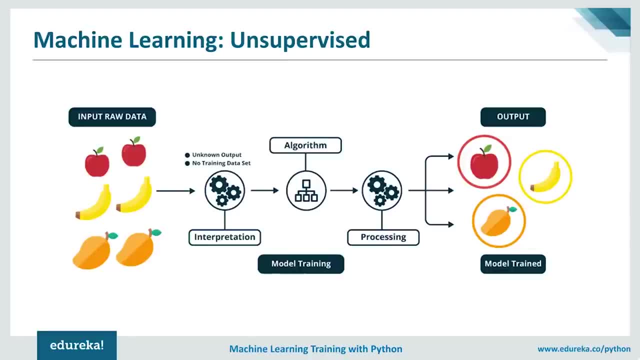 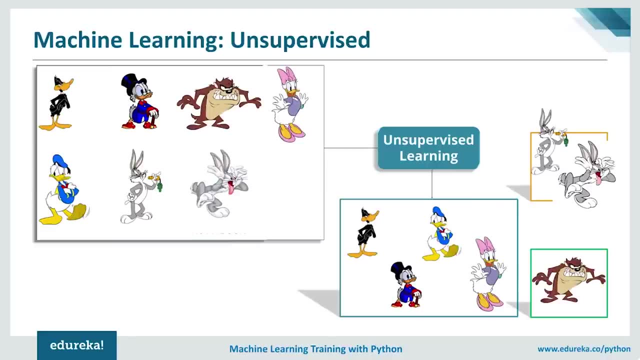 algorithm. The model will create clusters. on the basis of its training, It will group the similar fruits and make their cluster. Let me make things more clearer to you. Let's take another example of it. So in this slide, the image below shows an example. 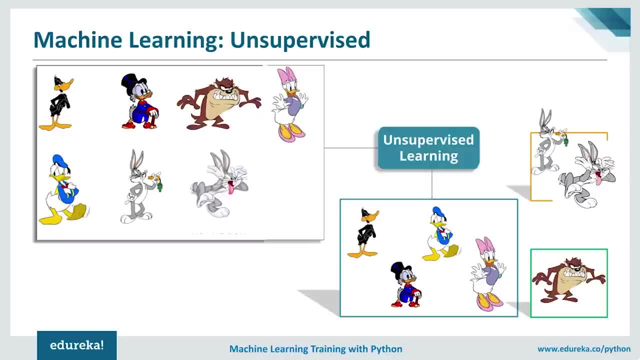 of unsupervised learning process. This algorithm processes an unlabeled training data set and, based on the characteristics, it groups the picture into three different clusters of data. despite the ability of grouping similar data into clusters, The algorithm is not capable to add labels to the group that will guard them only knows. 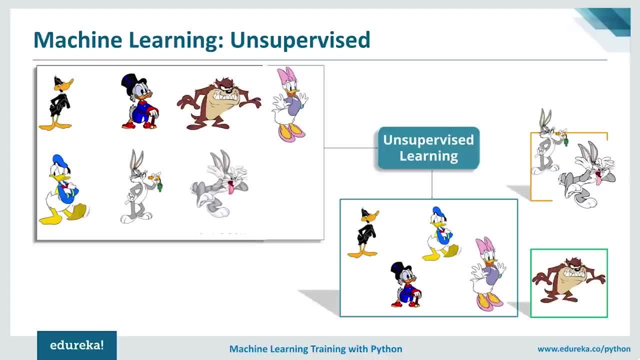 which data instances are similar, but it cannot identify the meaning of this group. So now you might be wondering why this category of machine learning is named as unsupervised learning. So these are called as unsupervised learning because, unlike supervised learning, ever. 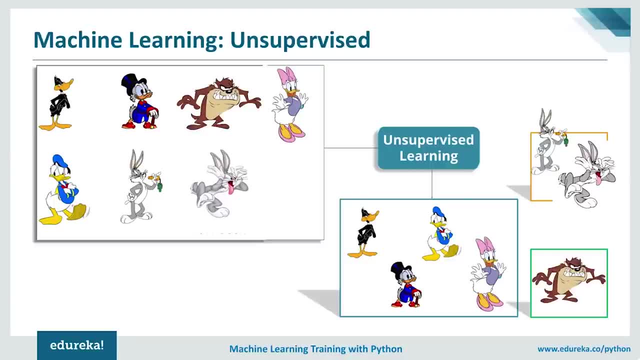 There are no correct answer and there is no teacher. algorithms are left on their own to discover and present the interesting structure in the data. Let's move on and see some of the popular unsupervised Learning algorithm. So we have here: K means a Peoria algorithm. 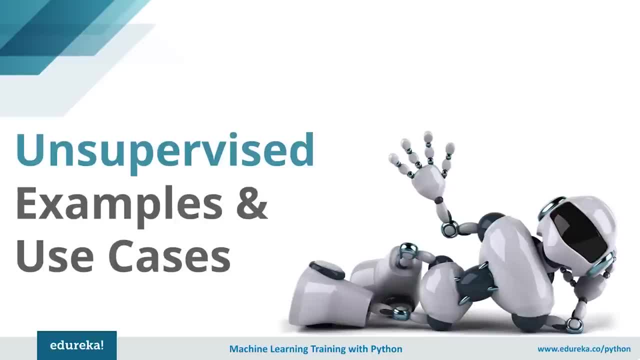 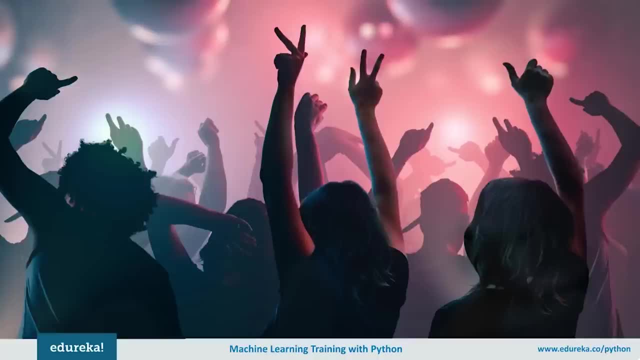 and hierarchical clustering. now let's move on and see some of the examples of unsupervised learning. suppose a friend invites you to his party and where you meet totally strangers. Now you will classify them using unsupervised learning, as you don't have any prior knowledge about them. 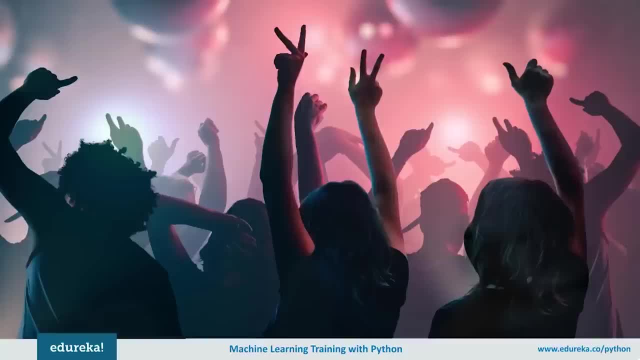 and this classification can be done on the basis of gender, age group, dressing, educational qualification or whatever way you might like. now why this learning is different from supervised learning. since you didn't use any past or prior knowledge about the people, you kept on classifying them on the go, as they kept on coming. 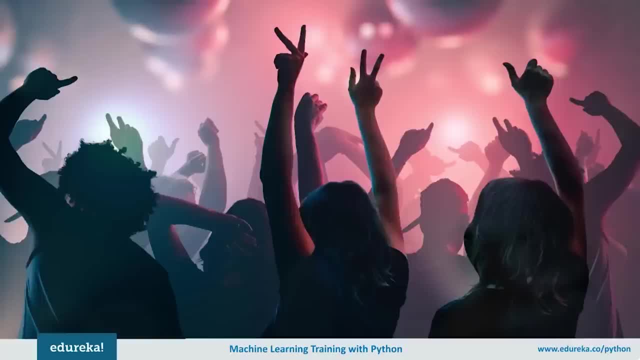 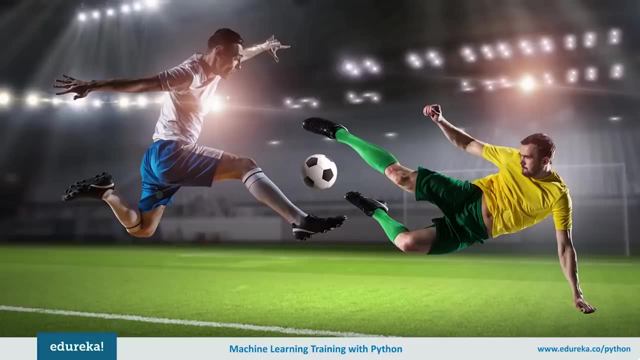 You kept on classifying them at: this category of people belong to this group, this category of people belong to that group, and so on. Okay, let's see one more example. Let's suppose you have never seen a football match before and by chance you watch a video on the internet. 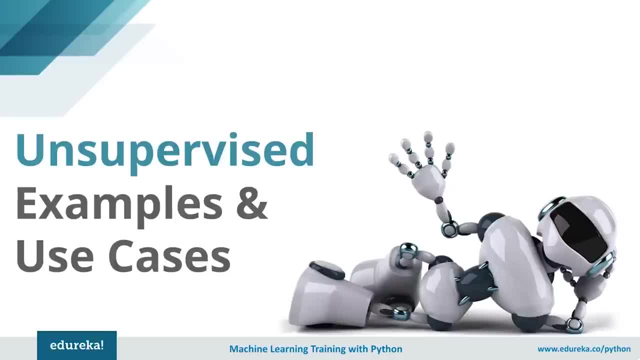 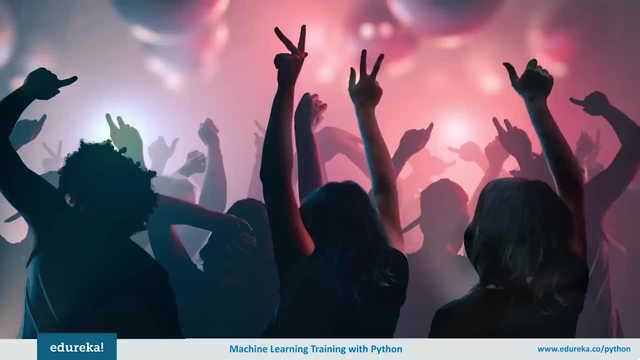 and hierarchical clustering. now let's move on and see some of the examples of unsupervised learning. suppose a friend invites you to his party and where you meet totally strangers. Now you will classify them using unsupervised learning, as you don't have any prior knowledge about them. 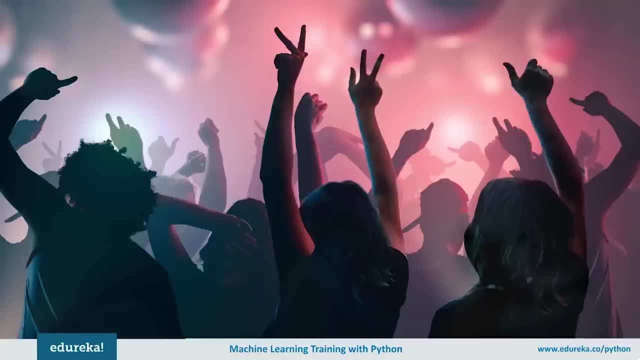 and this classification can be done on the basis of gender, age group, dressing, educational qualification or whatever way you might like. now why this learning is different from supervised learning. since you didn't use any past or prior knowledge about the people, you kept on classifying them on the go, as they kept on coming. 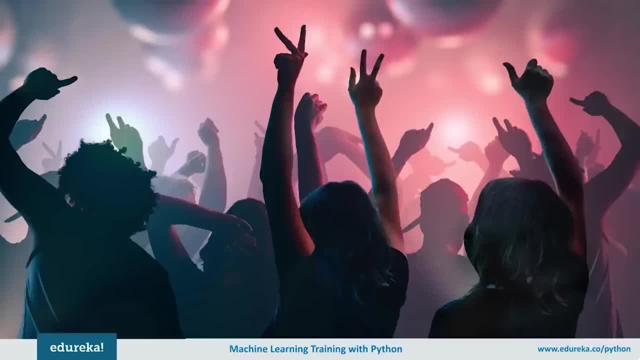 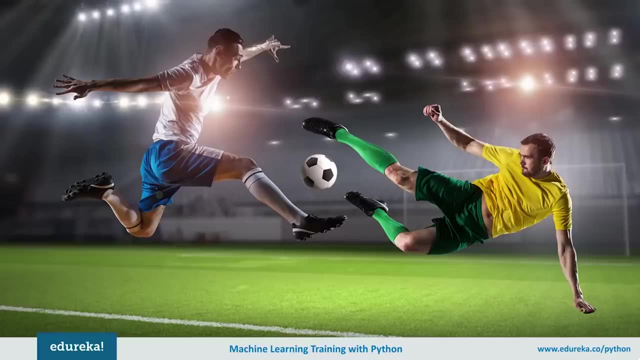 You kept on classifying them at: this category of people belong to this group, this category of people belong to that group, and so on. Okay, let's see one more example. Let's suppose you have never seen a football match before and by chance you watch a video on the internet. 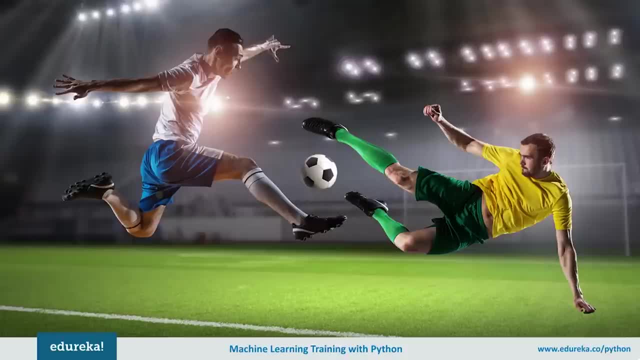 Now you can easily classify the players on the basis of different criterion, like player wearing the same kind of Jersey are in one class, player wearing different kind of Jersey are in different class. or you can classify them on the basis of their playing style. like the guys are attacker. 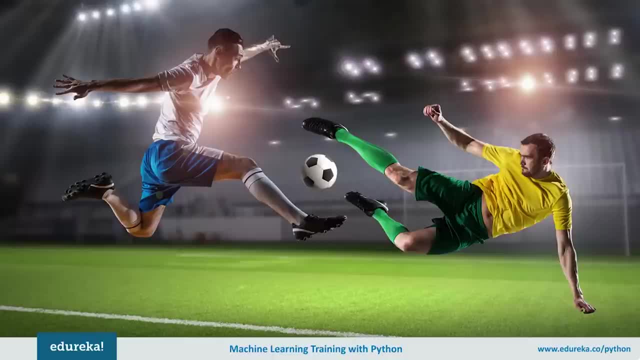 So he's in one class, He's a defender, He's in another class, or you can classify them whatever way you observe the things. So this was also an example of unsupervised learning. Let's move on and see how unsupervised learning is used. 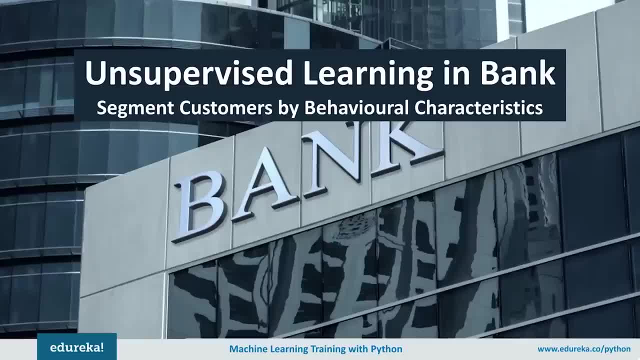 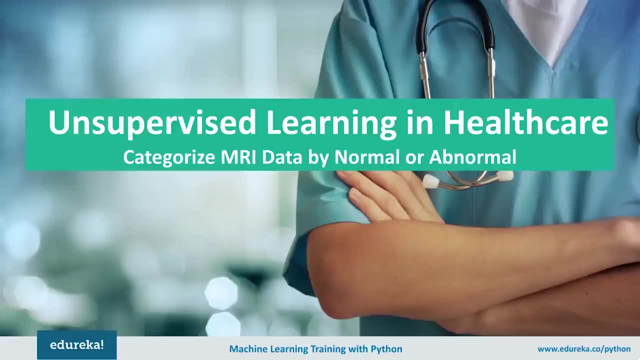 in the sectors of banking, healthcare and retail. So starting with banking sector. so in banking sector, it is used to segment customers by behavioral characteristic, by surveying prospects and customers, to develop multiple segments using clustering. and healthcare sector It is used to categorize the MRA data by normal 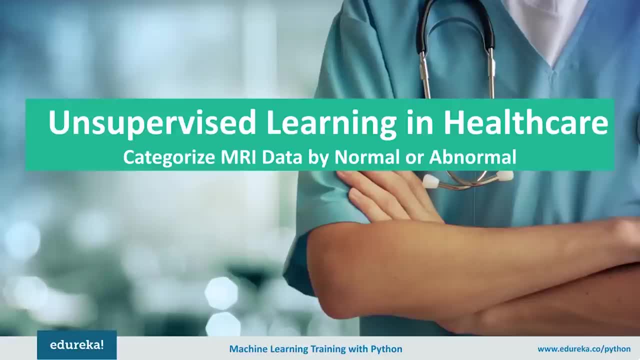 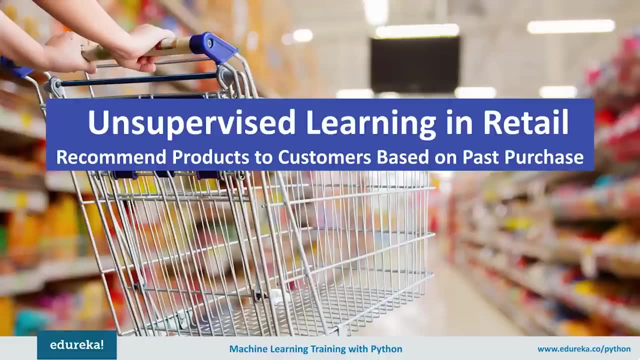 or abnormal images. it uses deep learning techniques to build a model that learns from different features of images to recognize a different pattern. next, as the retail sector. in retail sector, It is used to recommend the products to customer based on their past purchases. it does this by building a collaborative filtering model based. 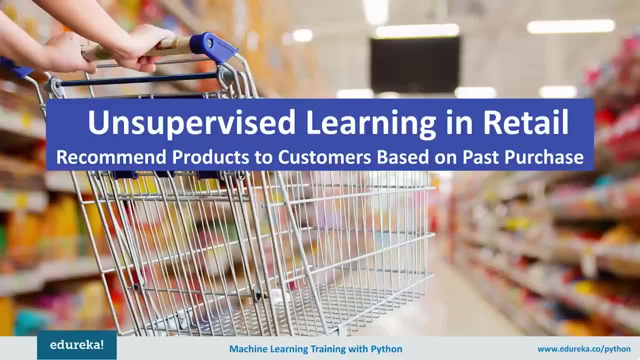 on the past purchases by them. I assume you guys now have a proper idea of what unsupervised learning means. if you have any slightest doubt, don't hesitate and add your doubt to the comment section. So let's discuss the third and the last type. 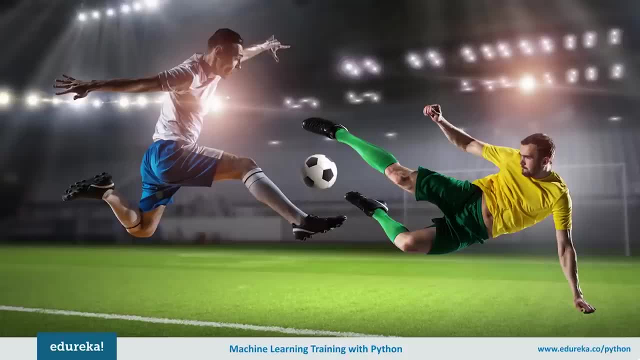 Now you can easily classify the players on the basis of different criterion, like player wearing the same kind of Jersey are in one class, player wearing different kind of Jersey are in different class. or you can classify them on the basis of their playing style. like the guys are attacker. 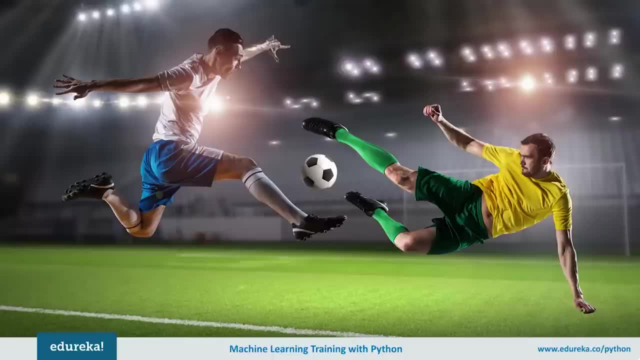 So he's in one class, He's a defender, He's in another class, or you can classify them whatever way you observe the things. So this was also an example of unsupervised learning. Let's move on and see how unsupervised learning is used. 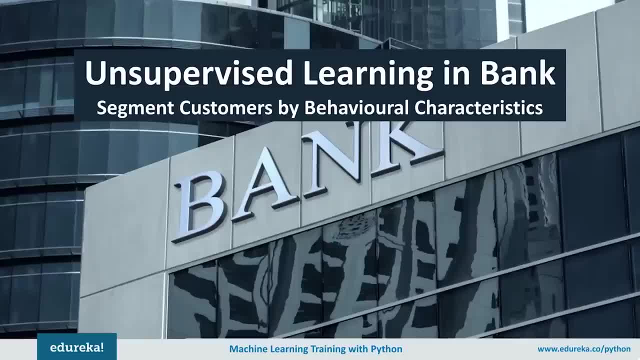 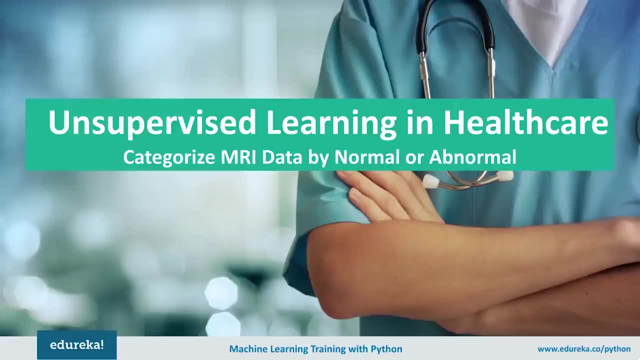 in the sectors of banking, healthcare and retail. So starting with banking sector. so in banking sector, it is used to segment customers by behavioral characteristic, by surveying prospects and customers, to develop multiple segments using clustering. and healthcare sector It is used to categorize the MRA data by normal 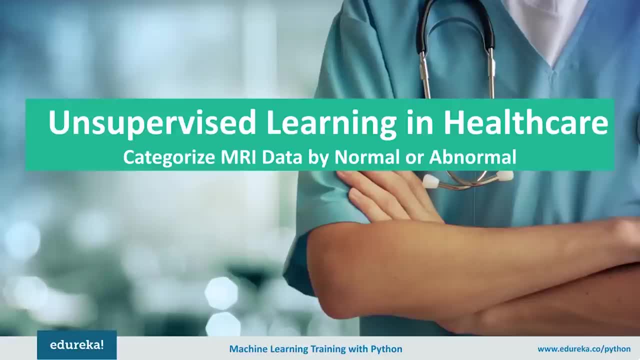 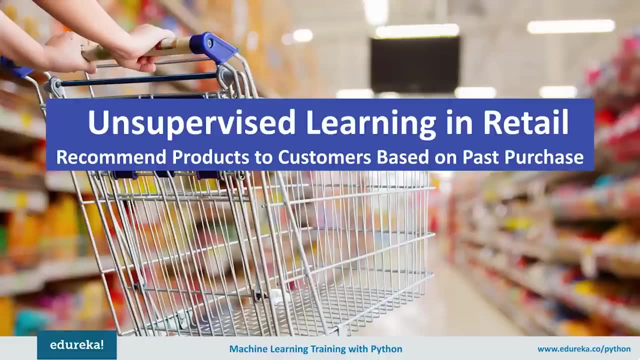 or abnormal images. it uses deep learning techniques to build a model that learns from different features of images to recognize a different pattern. next is the retail sector. in retail sector, It is used to recommend the products to customer based on their past purchases. It does this by building a collaborative filtering model based. 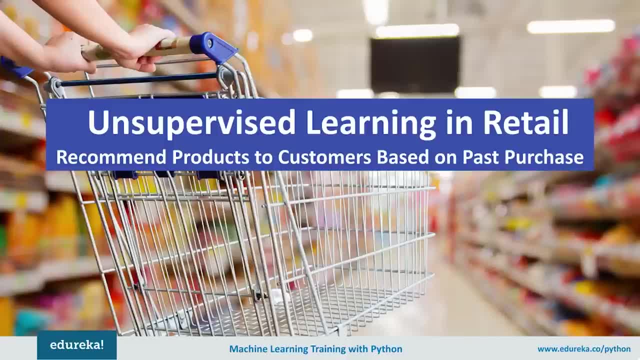 on the past purchases by them. I assume you guys now have a proper idea of what unsupervised learning means. if you have any slightest doubt, don't hesitate and add your doubt to the comment section. So let's discuss the third and the last type. 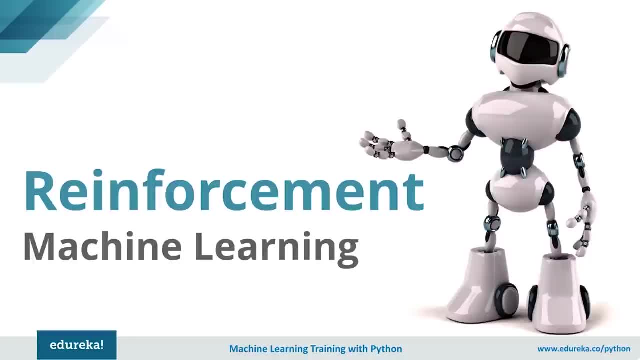 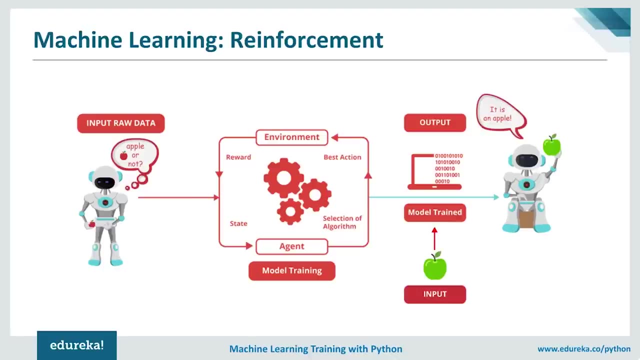 of machine learning, that is, reinforcement learning. So what is reinforcement learning? Well, reinforcement learning is a type of machine learning algorithm which allows software agents and machine to automatically determine the ideal behavior within a specific context to maximize its performance. The reinforcement learning is about interaction. 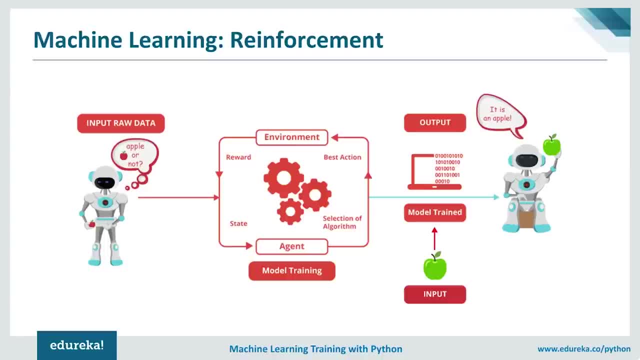 between two elements: the environment and the learning agent. the learning agent leverages to mechanism, namely exploration and exploitation. when learning agent acts on trial and error basis, It is termed as exploration, and when it acts based on the knowledge gained from the environment, It is referred to as exploitation. 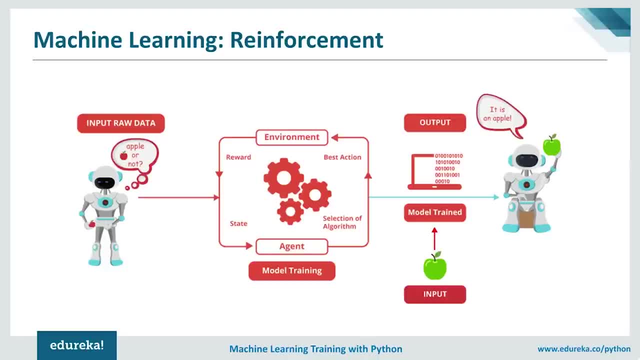 and this environment rewards the agent for correct actions, which is reinforcement signal. leveraging the rewards obtained, the agent It proves its environment knowledge to select the next action. in this image You can see that the machine is confused, whether it is an apple or it's not an apple. 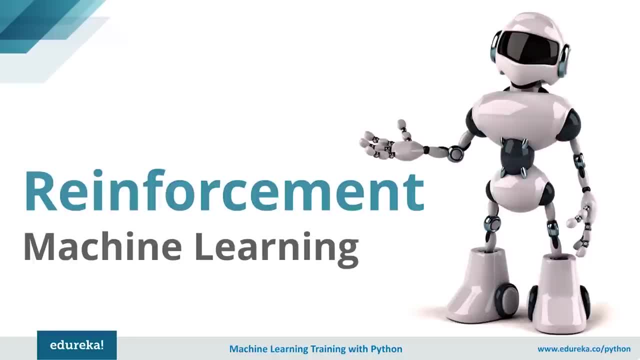 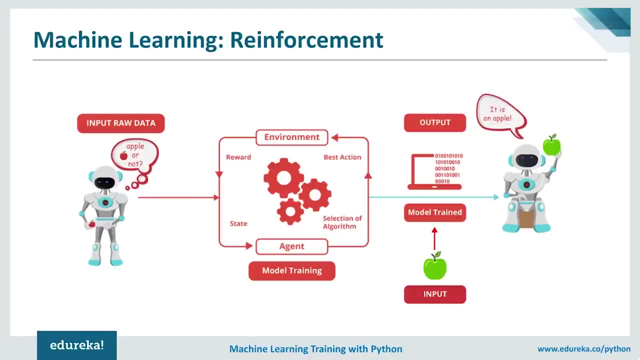 of machine learning, that is, reinforcement learning. So what is reinforcement learning? Well, reinforcement learning is a type of machine learning algorithm which allows software agents and machine to automatically determine the ideal behavior within a specific context to maximize its performance. The reinforcement learning is about interaction. 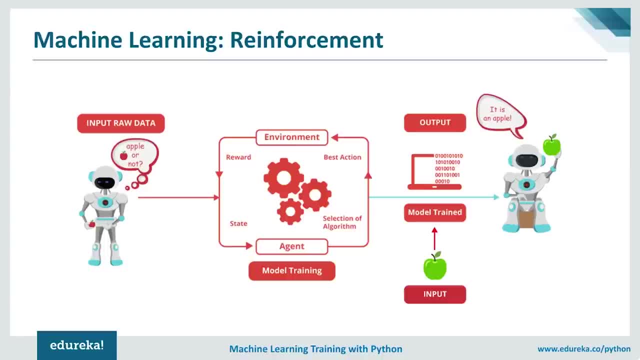 between two elements: the environment and the learning agent. the learning agent leverages to mechanism, namely exploration and exploitation. when learning agent acts on trial and error basis, It is termed as exploration, and when it acts based on the knowledge gained from the environment, It is referred to as exploitation. 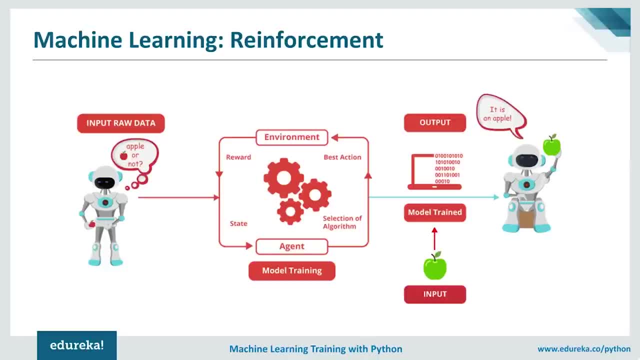 and this environment rewards the agent for correct actions, which is reinforcement signal. leveraging the rewards obtained, the agent It proves its environment knowledge to select the next action. in this image You can see that the machine is confused, whether it is an apple or it's not an apple. 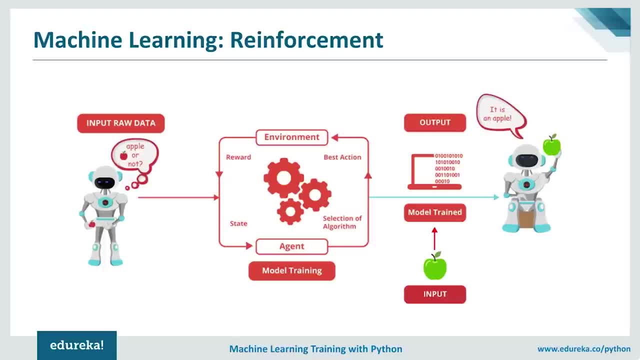 Then the machine is trained using reinforcement learning. if it makes correct decision, it get rewards point for it, and in case of wrong it gets a penalty for that. once the training is done, Now the machine can easily identify which one of them is an apple. Let's see an example here. 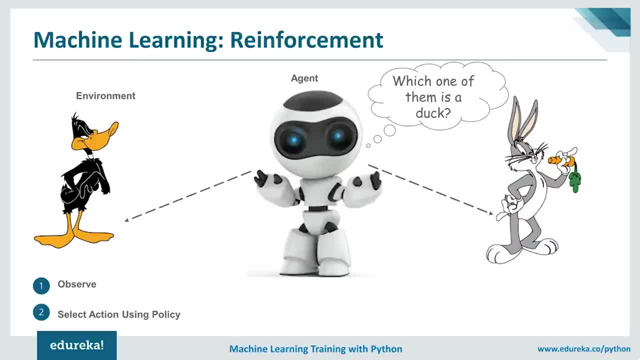 We can see that we have. an agent was, to judge from the environment, to find out which of the two is a duck. The first task he did is to observe the environment, next to select some action using some policy. It seems that the machine has made a wrong decision. 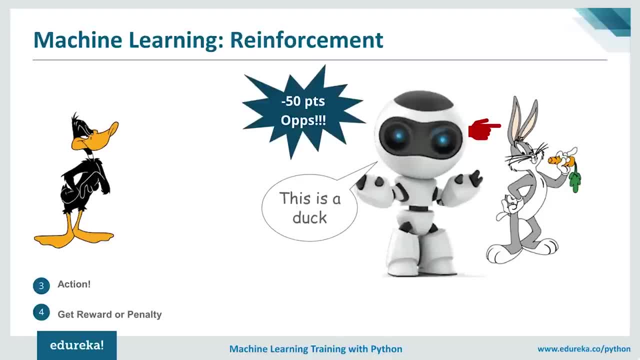 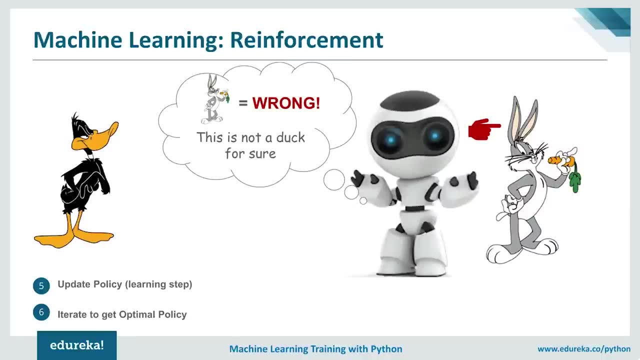 by choosing a bunny as a duck. So the machine will get penalty for it. For example, minus 50 point for a wrong answer. right now The machine will update its policy and this will continue till the machine gets an optimal policy. from the next time machine will know that bunny is not a duck. 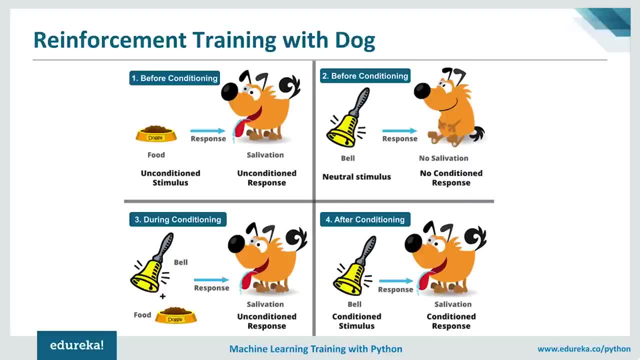 Let's see some of the use cases of reinforcement learning, but before that, let's see how Pavlo trained his dog using reinforcement learning, or how he applied the reinforcement method to train his dog. Pavlo integrated learning in four stages. Initially, Pavlo gave meat to his dog. 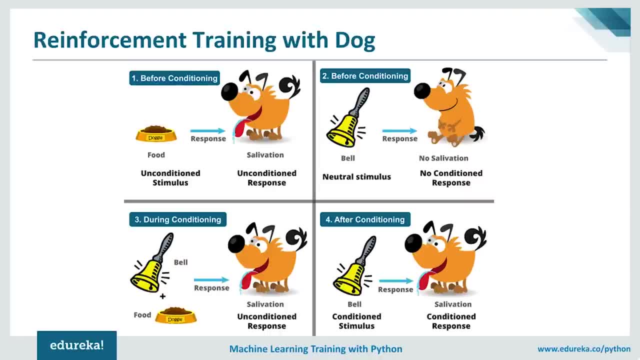 and in response to the meat, the dog started salivating. next what he did? he created a sound with the bell. for this the dog did not respond anything. in the third part He tried to condition the dog by using the bell and then giving him the food. seeing the food, 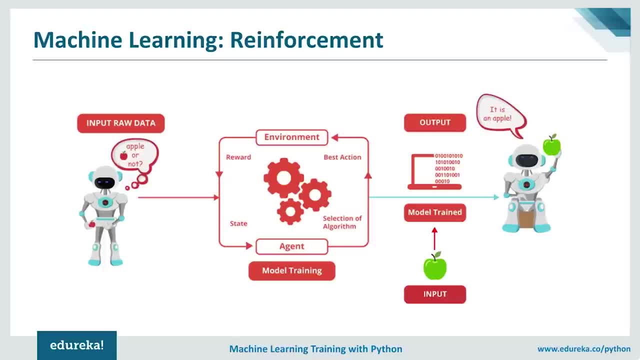 Then the machine is trained using reinforcement learning. if it makes correct decision, it get rewards point for it, and in case of wrong it gets a penalty for that. once the training is done, Now the machine can easily identify which one of them is an apple. Let's see an example here. 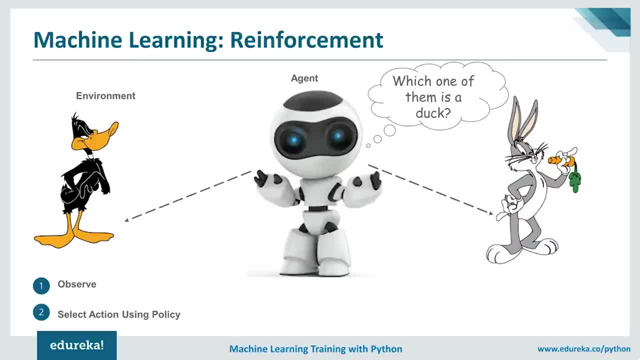 We can see that we have. an agent was, to judge from the environment, to find out which of the two is a duck. The first task he did is to observe the environment, next to select some action using some policy. It seems that the machine has made a wrong decision. 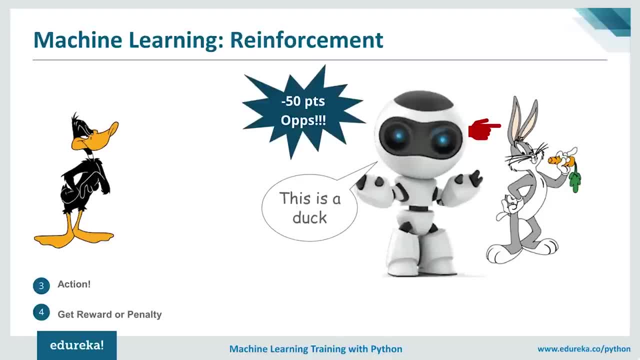 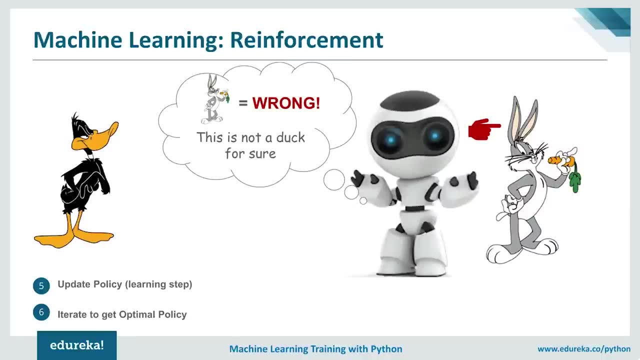 by choosing a bunny as a duck. So the machine will get penalty for it. For example, minus 50 point for a wrong answer. right now The machine will update its policy and this will continue till the machine gets an optimal policy. from the next time machine will know that bunny is not a duck. 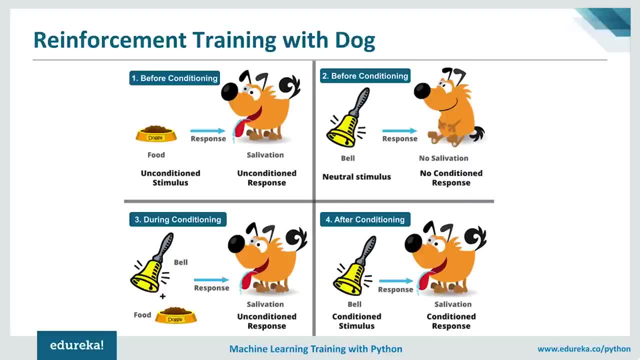 Let's see some of the use cases of reinforcement learning, but before that, let's see how Pavlo trained his dog using reinforcement learning, or how he applied the reinforcement method to train his dog. Pavlo integrated learning in four stages. Initially, Pavlo gave meat to his dog. 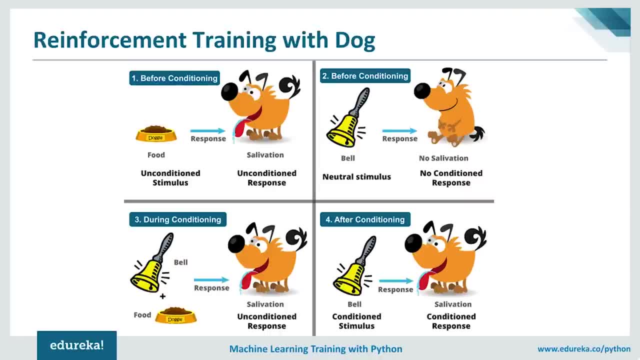 and in response to the meat, the dog started salivating. next what he did? he created a sound with the bell. for this the dog did not respond anything. in the third part He tried to condition the dog by using the bell and then giving him the food. seeing the food, 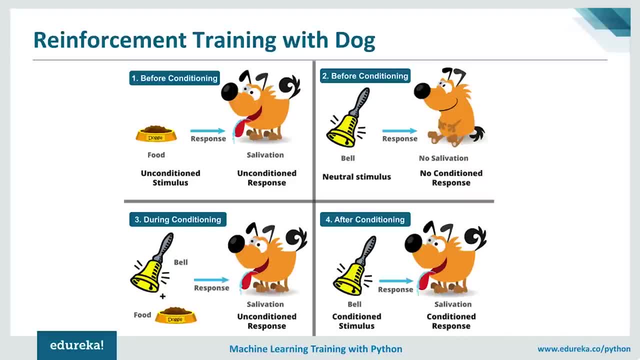 The dog started salivating. eventually, a situation came when the dog started salivating just after hearing the bell, even if the food was not given to him, as the dog was reinforced that whenever the master will ring the bell, he will get the food. now, 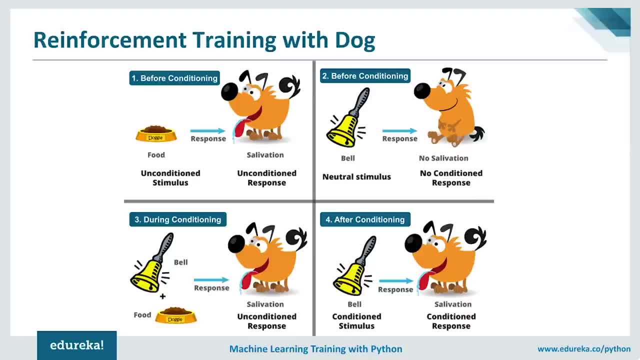 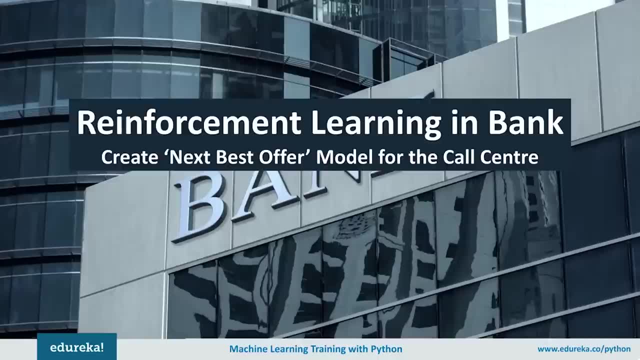 let's move on and see how reinforcement learning is applied in the field of banking, healthcare and retail sector. So, starting with the banking sector and banking sector, reinforcement learning is used to create a next best offer model for a call center by building a predictive model that learns over time as user accept or reject offer made. 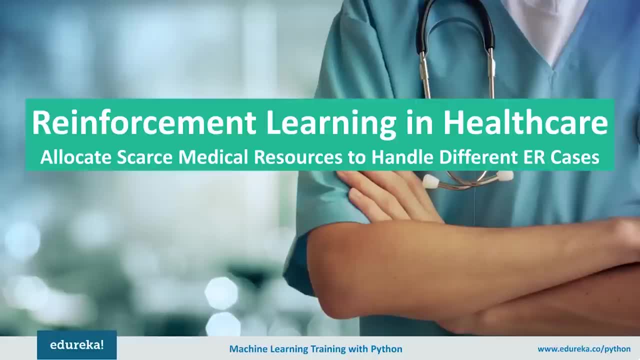 by the sales staff. fine. now in healthcare sector, It is used to allocate the scars medical resources to handle different type of ER cases by building a mark of decision process that learns treatment strategies for each type of ER case. next and the last, comes the retail sector. 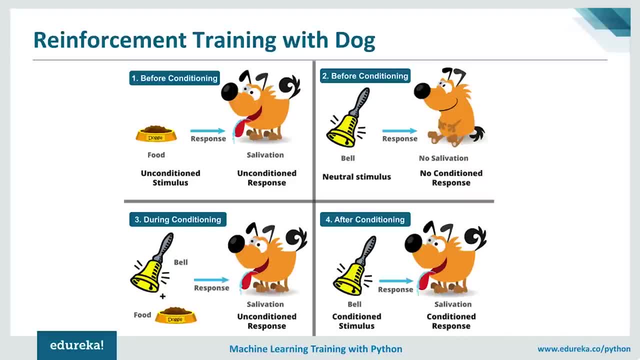 The dog started salivating. eventually, a situation came when the dog started salivating just after hearing the bell, even if the food was not given to him, as the dog was reinforced that whenever the master will ring the bell, he will get the food. now, 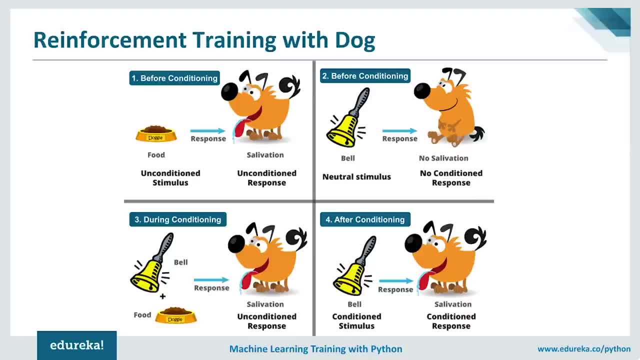 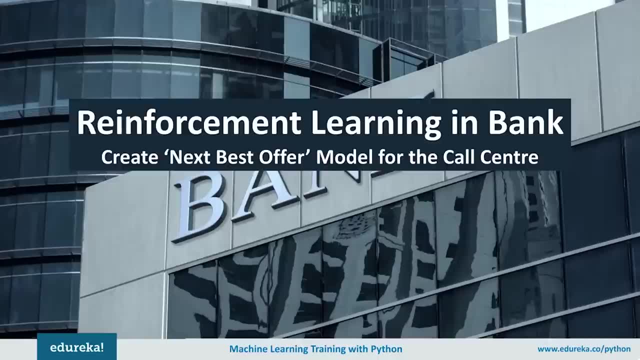 let's move on and see how reinforcement learning is applied in the field of banking, healthcare and retail sector. So, starting with the banking sector and banking sector, reinforcement learning is used to create a next best offer model for a call center by building a predictive model that learns over time as user accept or reject offer made. 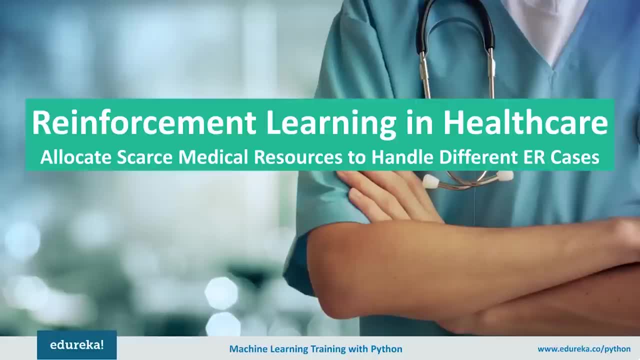 by the sales staff. fine. now in healthcare sector, It is used to allocate the scars medical resources to handle different type of ER cases by building a mark of decision process that learns treatment strategies for each type of ER case. next and the last, comes the retail sector. 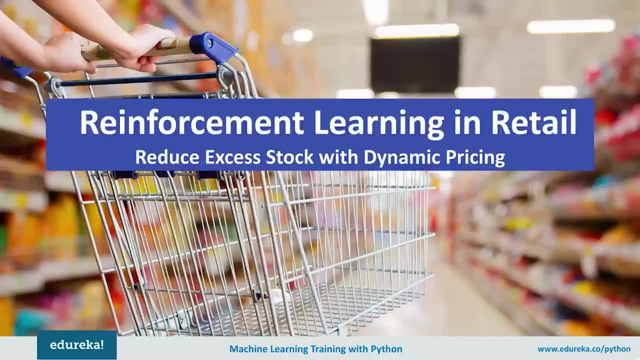 So let's see how reinforcement learning is applied to retail sector. in retail sector It can be used to reduce excess stock with dynamic pricing by building a dynamic pricing model that adjust the price based on customer response to the offers. I hope by now you have attained some understanding. 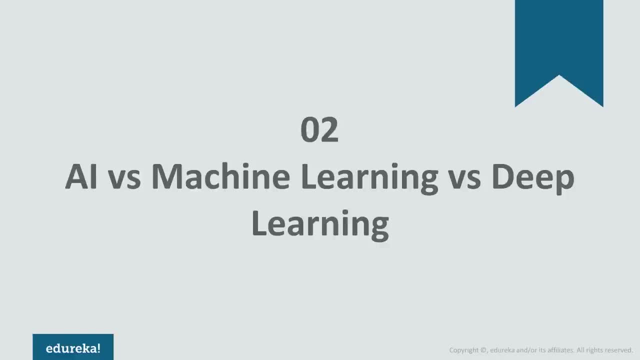 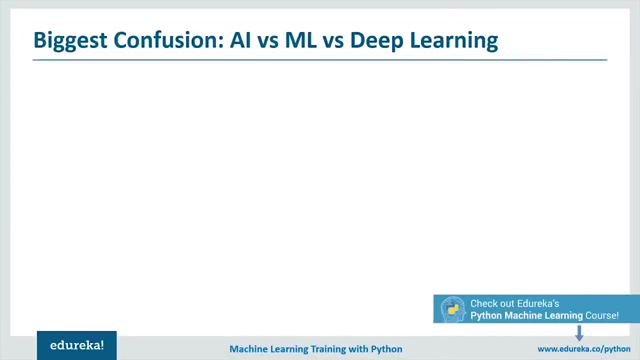 of what is machine learning and you are ready to move ahead. Welcome to today's topic of discussion on AI versus machine learning, versus deep learning. These are the term which have confused a lot of people, and if you two are one among them, let me resolve it for you. 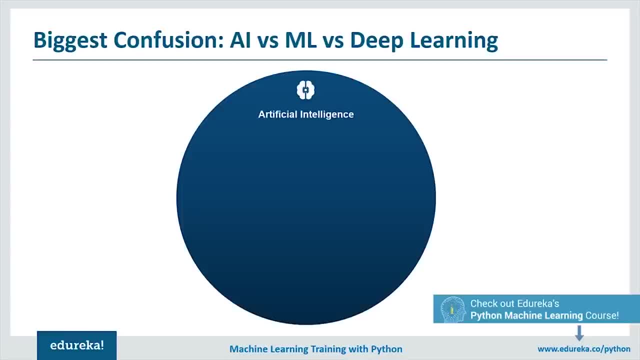 Well, artificial intelligence is a broader Umbrella under which machine learning and deep learning come. You can also see in the diagram that even deep learning is a subset of machine learning. So you can say that all three of them- the AI, the machine learning and deep learning- are just the subset of each other. 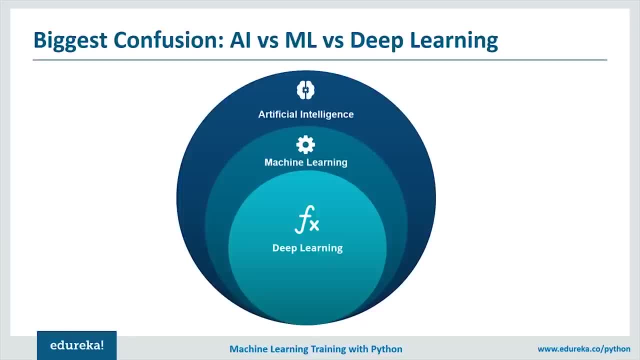 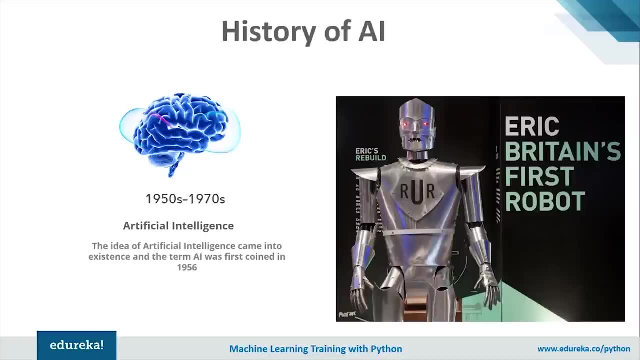 So let's move on and understand how exactly the differ from each other. So let's start with artificial intelligence. The term artificial intelligence was first coined in the year 1956. The concept is pretty old, but it has gained its popularity recently. 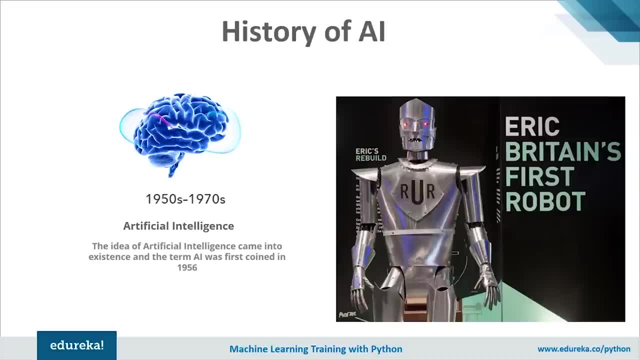 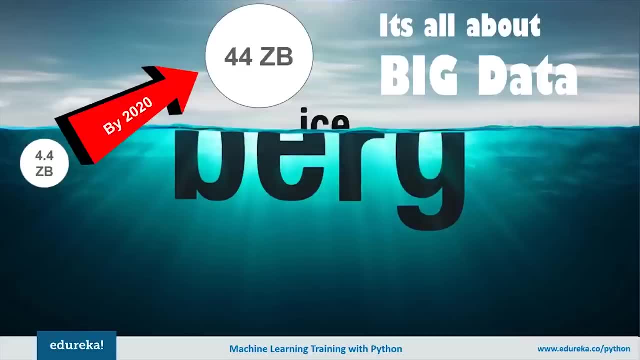 but why? well, the reason is: earlier We had very small amount of data. The data we had was not enough to predict the accurate result. But now there's a tremendous increase in the amount of data. statistics suggest that by 2020, the accumulated volume of data will increase. 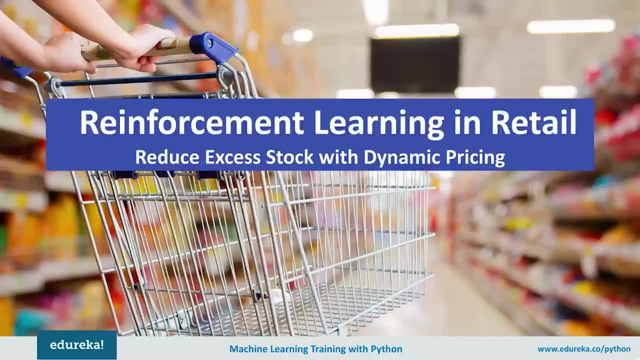 So let's see how reinforcement learning is applied to retail sector. in retail sector It can be used to reduce excess stock with dynamic pricing by building a dynamic pricing model that adjust the price based on customer response to the offers. I hope by now you have attained some understanding. 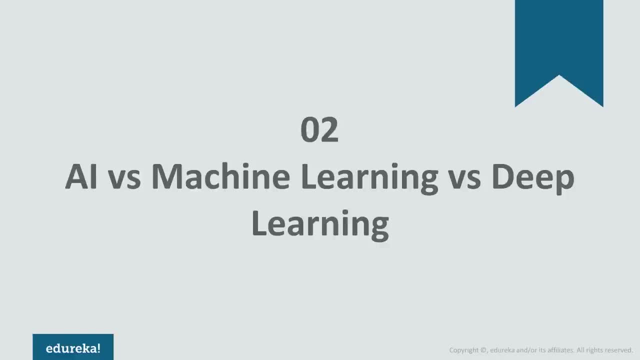 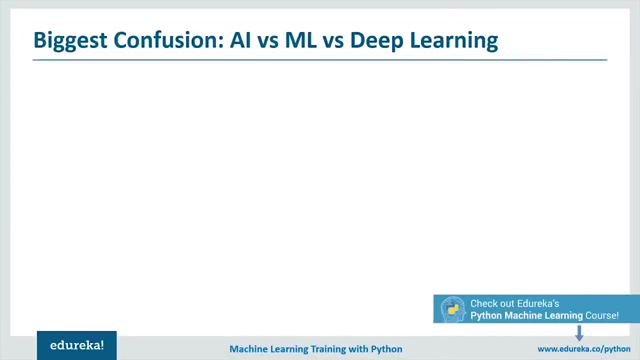 of what is machine learning and you are ready to move ahead. Welcome to today's topic of discussion on AI versus machine learning, versus deep learning. These are the term which have confused a lot of people, and if you two are one among them, let me resolve it for you. 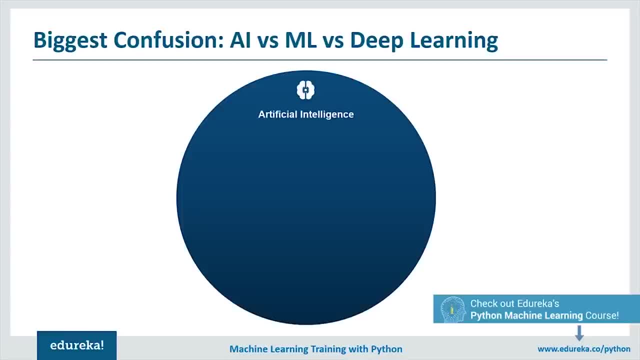 Well, artificial intelligence is a broader Umbrella under which machine learning and deep learning come. You can also see in the diagram that even deep learning is a subset of machine learning. So you can say that all three of them- the AI, the machine learning and deep learning- are just the subset of each other. 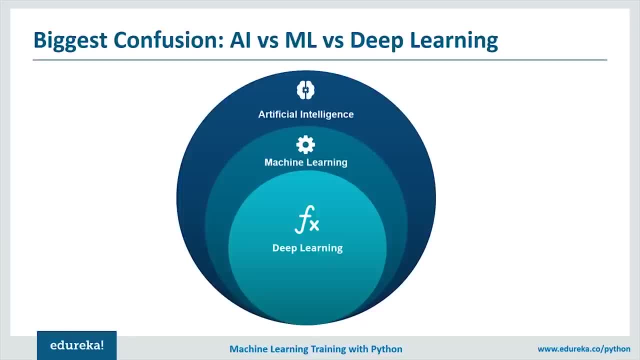 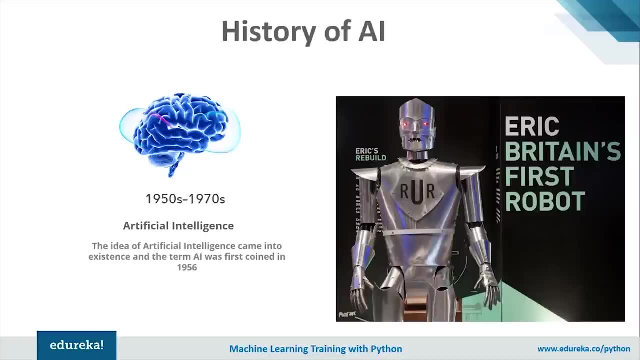 So let's move on and understand how exactly the differ from each other. So let's start with artificial intelligence. The term artificial intelligence was first coined in the year 1956. The concept is pretty old, but it has gained its popularity recently. 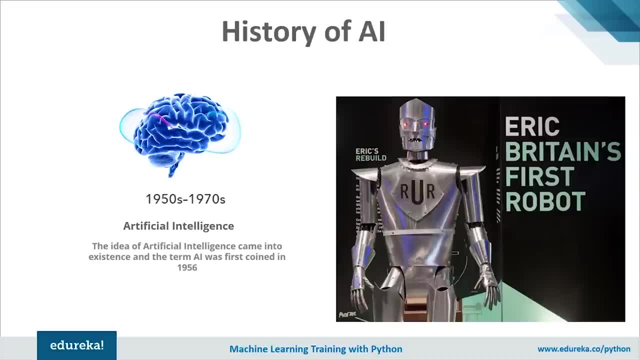 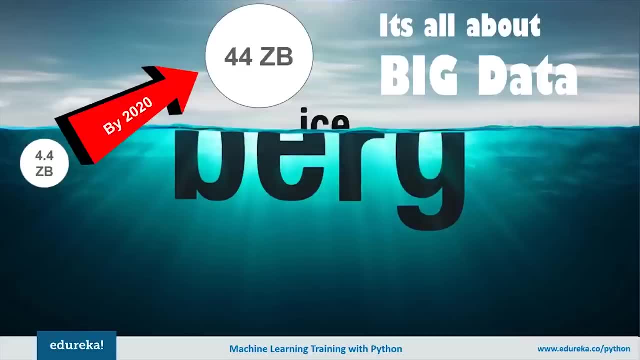 but why? well, the reason is: earlier We had very small amount of data. The data we had was not enough to predict the accurate result. But now there's a tremendous increase in the amount of data. statistics suggest that by 2020, the accumulated volume of data will increase. 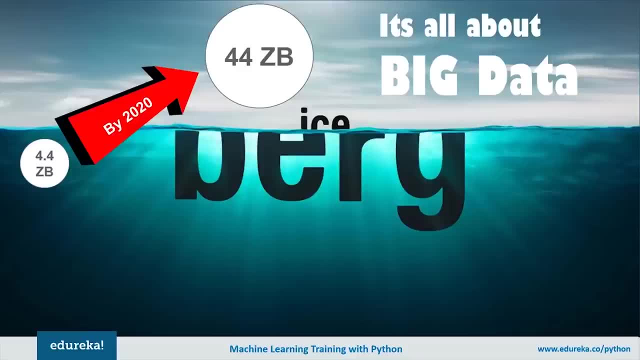 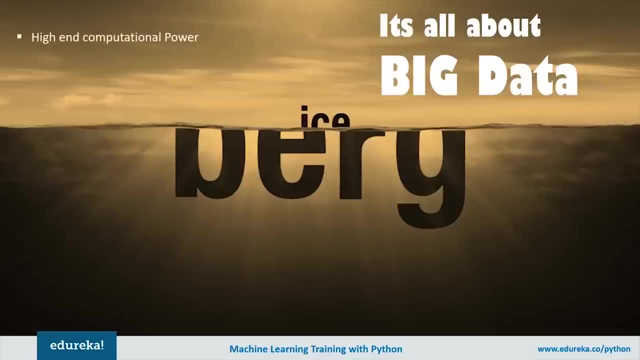 from 4.4 zettabytes to roughly around 44 zettabytes, or 44 trillion GBs of data. Along with such enormous amount of data, Now we have more advanced algorithm and high-end computing power and storage that can deal with such large amount of data. as a result, 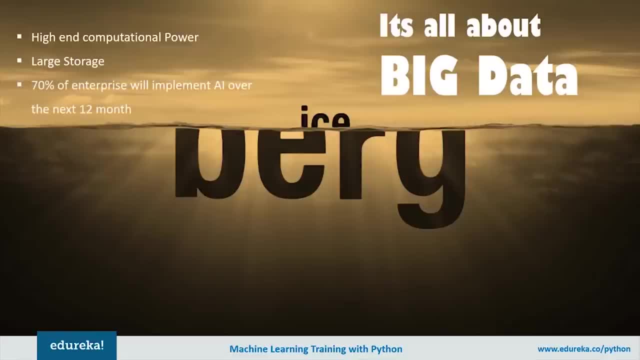 It is expected that 70% of Enterprise will implement AI over the next 12 months, which is up from 40% in 2016 and 51% in 2017. just for your understanding, What is AI? Well, it's nothing but a technique that enables the machine. 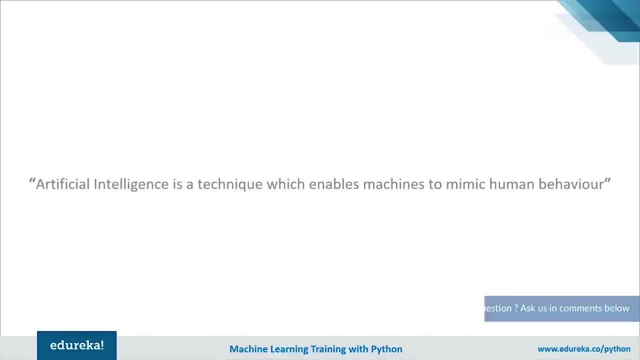 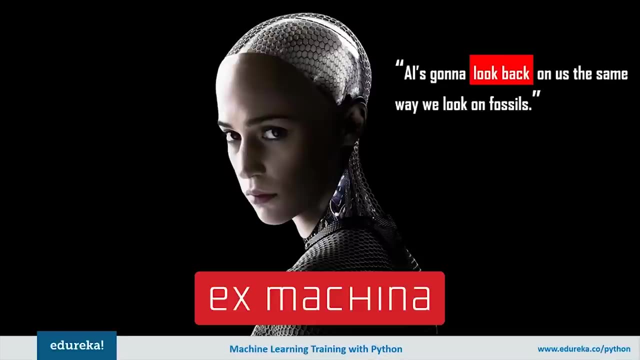 to act like humans by replicating the behavior and nature. with AI, It is possible for machine to learn from the experience. The machines adjust their responses based on new input, thereby performing human-like tasks. artificial intelligence can be trained to accomplish specific tasks by processing large amount of data. 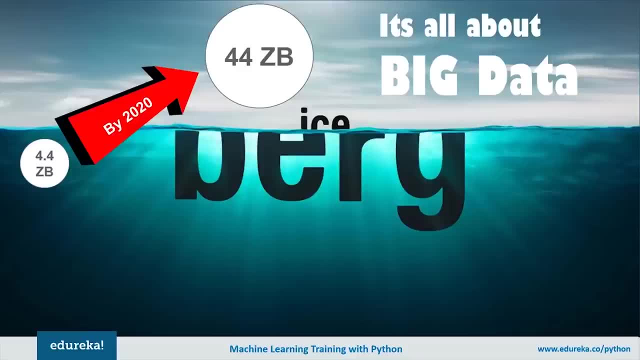 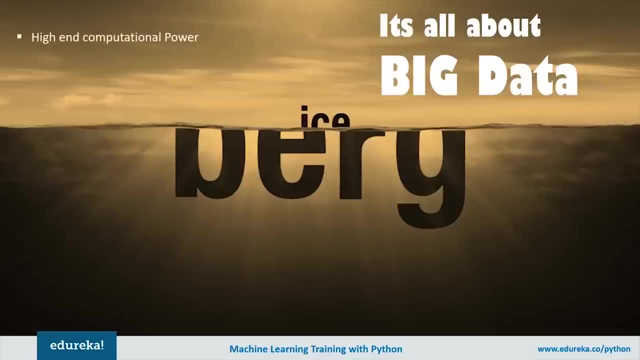 from 4.4 zettabytes to roughly around 44 zettabytes, or 44 trillion GBs of data. Along with such enormous amount of data, Now we have more advanced algorithm and high-end computing power and storage that can deal with such large amount of data. as a result, 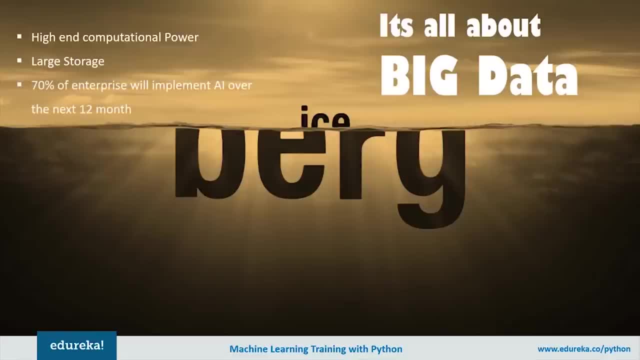 It is expected that 70% of Enterprise will implement AI over the next 12 months, which is up from 40% in 2016 and 51% in 2017. just for your understanding, What is AI? Well, it's nothing but a technique that enables the machine. 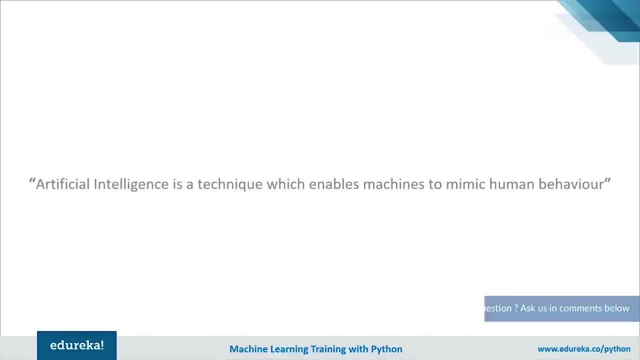 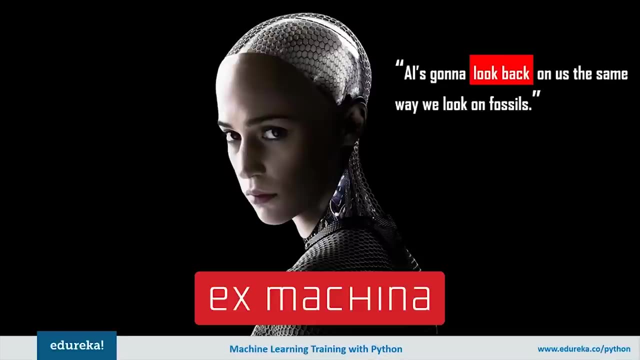 to act like humans by replicating the behavior and nature. with AI, It is possible for machine to learn from the experience. The machines adjust their responses based on new input, thereby performing human-like tasks. artificial intelligence can be trained to accomplish specific tasks by processing large amount of data. 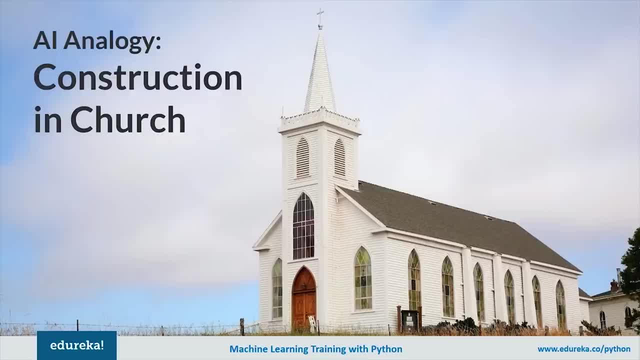 and recognizing pattern in them. You can consider that building an artificial intelligence is like building a church. the first church took generations to finish, So most of the workers who are working in it Never saw the final outcome. those working on it took pride in their crafts: building bricks. 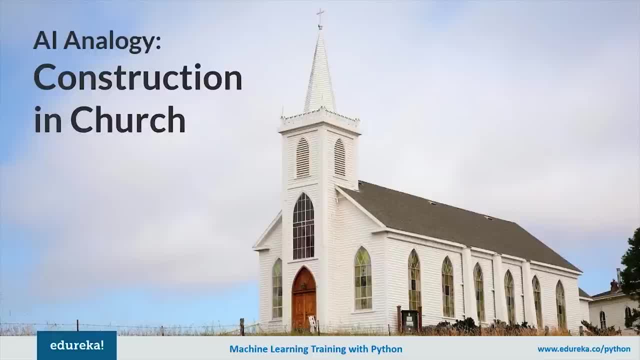 and chiseling stone that was going to be placed into the great structure. So, as AI researchers, we should think of ourselves as humble brick makers whose job is to study how to build components, example passes, planners or learning algorithm, or except, or anything that someday someone 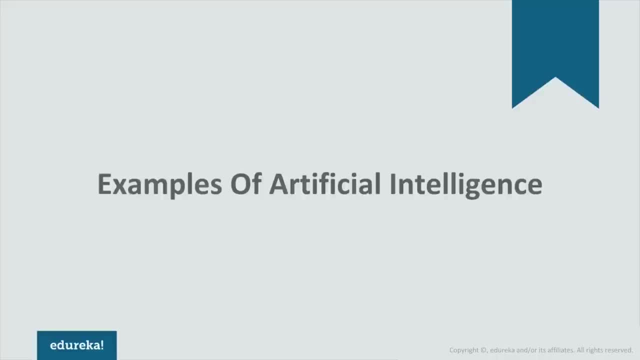 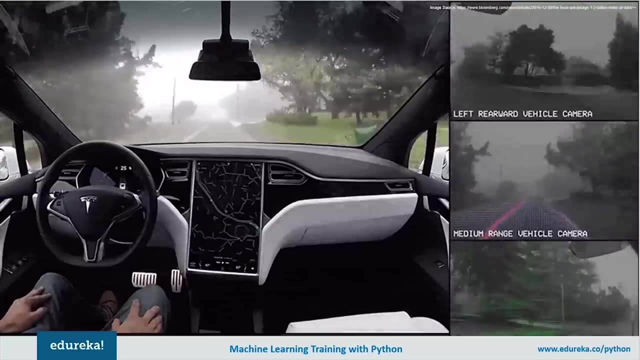 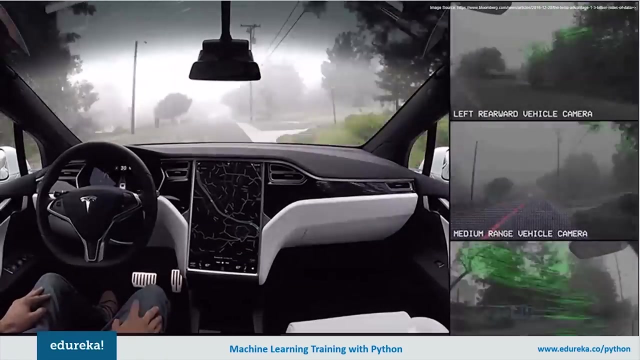 and somewhere will integrate into the intelligent systems. Some of the examples of artificial intelligence from our day-to-day life are Apple series Just playing computer, Tesla self-driving car and many more. these examples are based on deep learning and natural language processing. Well, this was about what is AI and how it gained its height. 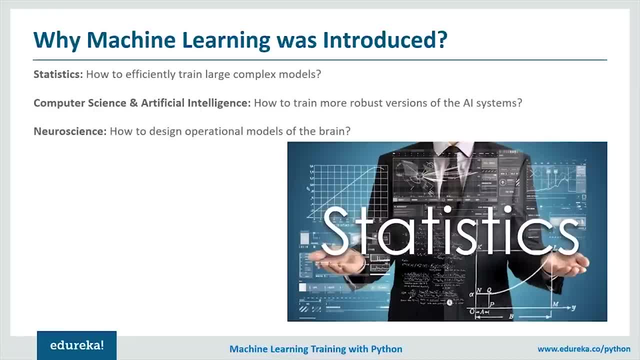 So, moving on ahead, Let's discuss about machine learning and see what it is and why it was even introduced. Well, machine learning came into existence in the late 80s and the early 90s, But what were the issues with the people which made the machine learning come into existence? 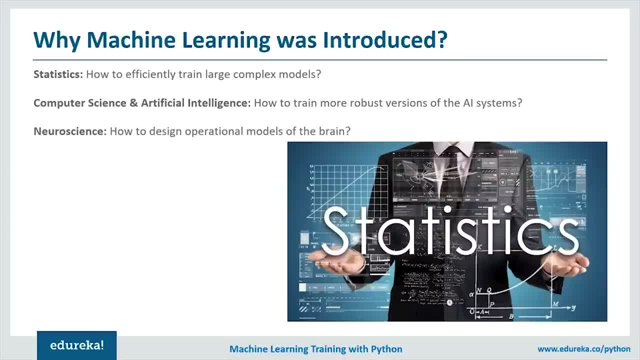 Let us discuss them one by one. In the field of statistics, The problem was how to efficiently train large, complex model. in the field of computer science and artificial intelligence, The problem was how to train more robust version of AI system, while in the case of neuroscience, problem faced 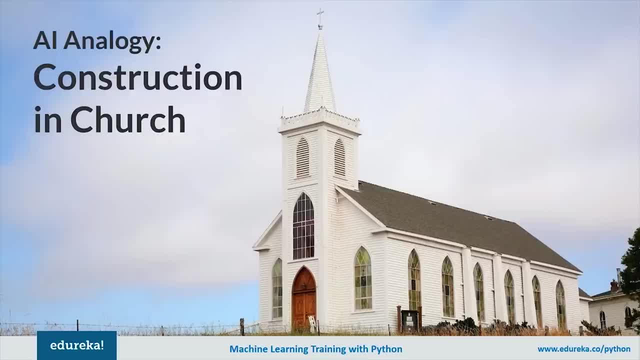 and recognizing pattern in them. You can consider that building an artificial intelligence is like building a church. the first church took generations to finish, So most of the workers who are working in it Never saw the final outcome. those working on it took pride in their crafts: building bricks. 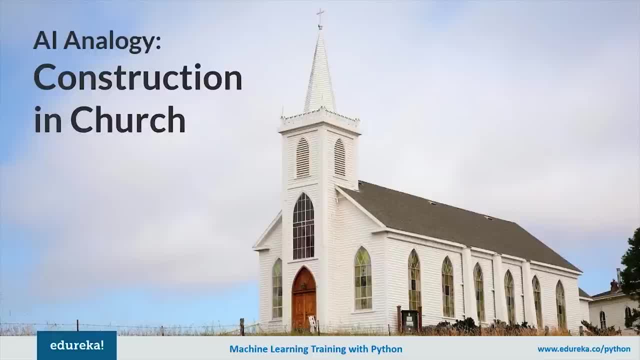 and chiseling stone that was going to be placed into the great structure. So, as AI researchers, we should think of ourselves as humble brick makers whose job is to study how to build components, example passes, planners or learning algorithm, or except, or anything that someday someone 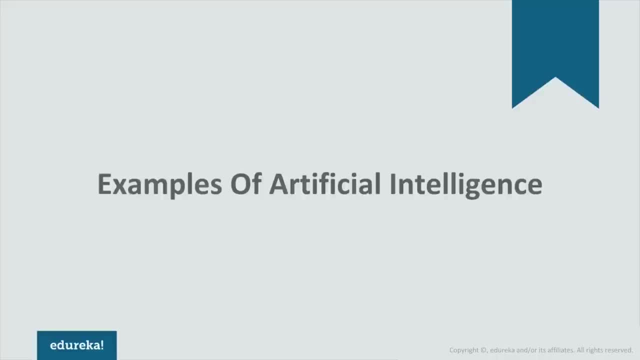 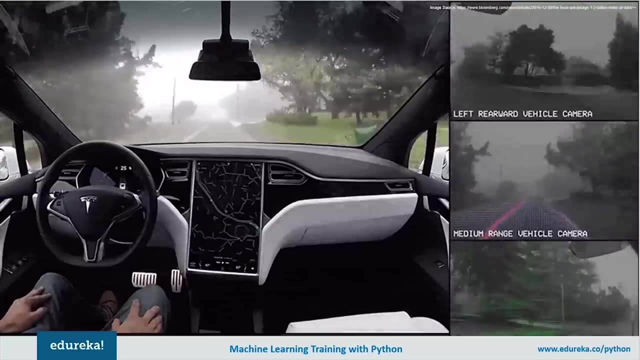 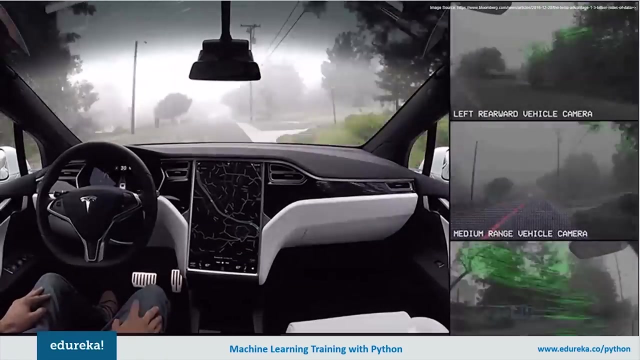 and somewhere will integrate into the intelligent systems. Some of the examples of artificial intelligence from our day-to-day life are Apple series Just playing computer, Tesla self-driving car and many more. these examples are based on deep learning and natural language processing. Well, this was about what is AI and how it gained its height. 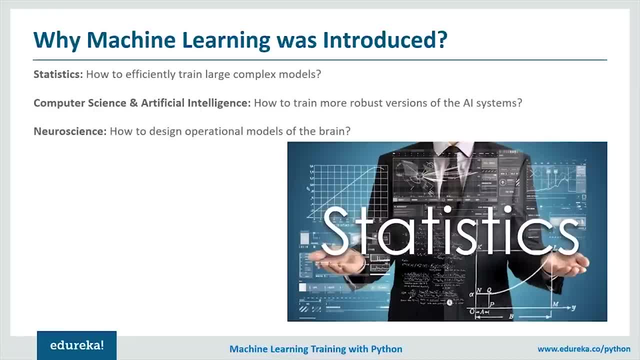 So, moving on ahead, Let's discuss about machine learning and see what it is and why it was even introduced. Well, machine learning came into existence in the late 80s and the early 90s, But what were the issues with the people which made the machine learning come into existence? 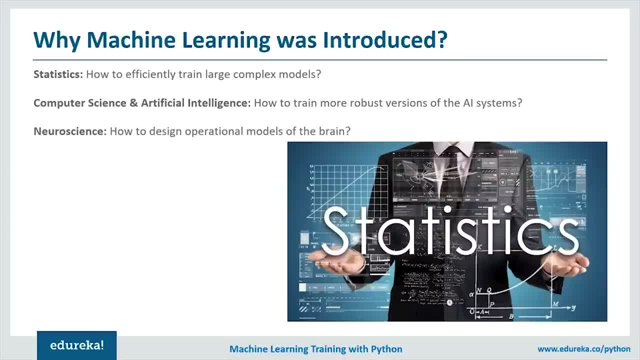 Let us discuss them one by one. In the field of statistics, The problem was how to efficiently train large, complex model. in the field of computer science and artificial intelligence, The problem was how to train more robust version of AI system, while in the case of neuroscience, problem faced 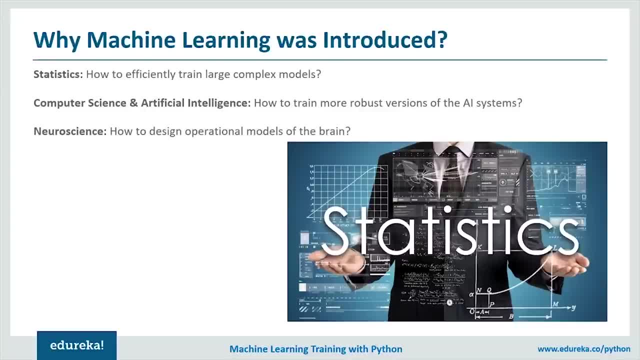 by the researchers was how to design operational model of the brain. So these were some of the issues which had the largest influence and led to the existence of the machine learning. now, this machine learning shifted its focus from the symbolic approaches it had inherited from the AI. 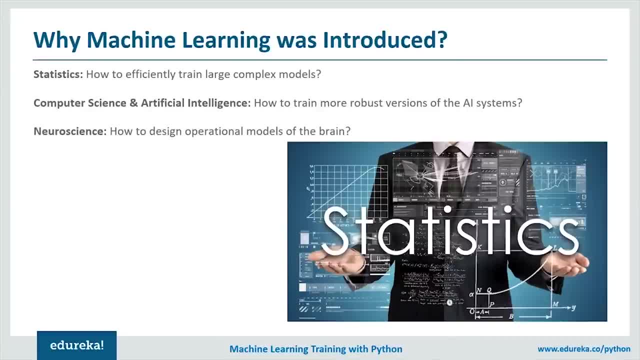 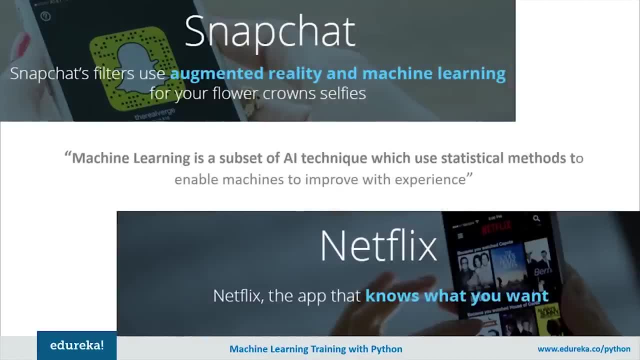 and move towards the methods and model It had bought from statistics and probability theory. So let's proceed and see what exactly is machine learning. Well, machine learning is a subset of AI which enables the computer to act and make data-driven decisions to carry out a certain task. 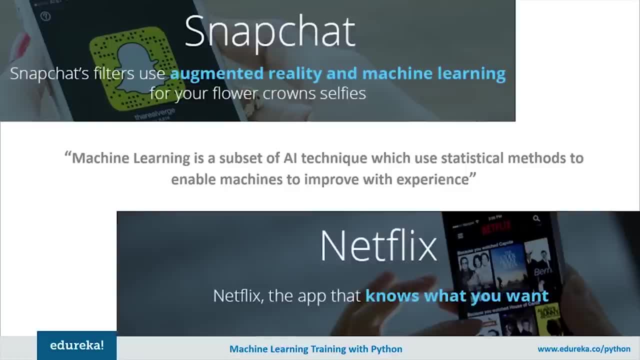 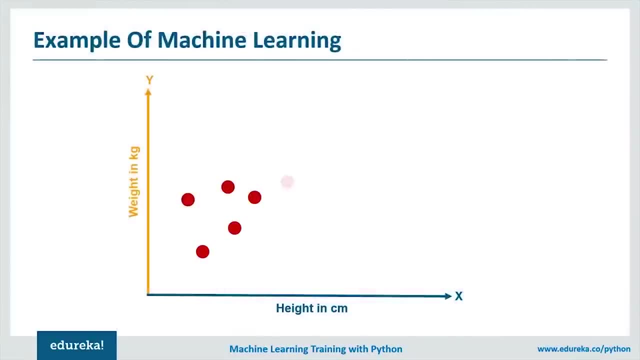 These programs or algorithms are designed in a way that they can learn and improve over time when exposed to new data. Let's see an example of machine learning. Let's say you want to create a system which tells the expected weight of a person based on its height. 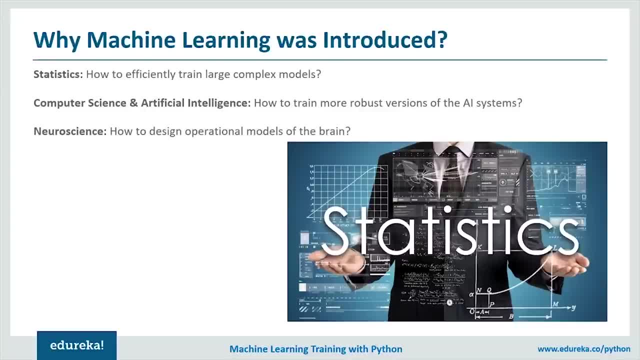 by the researchers was how to design operational model of the brain. So these were some of the issues which had the largest influence and led to the existence of the machine learning. now, this machine learning shifted its focus from the symbolic approaches it had inherited from the AI. 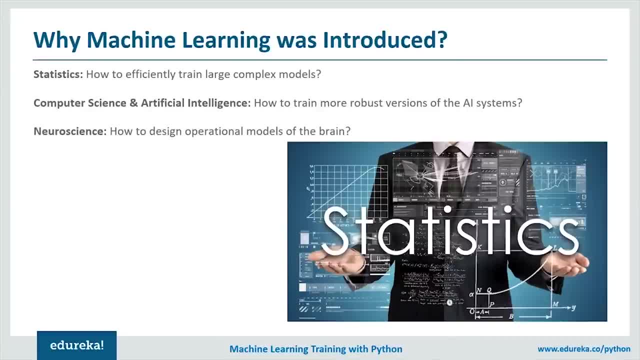 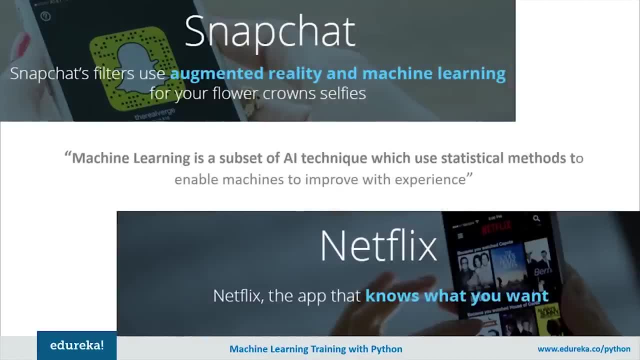 and move towards the methods and model It had bought from statistics and probability theory. So let's proceed and see what exactly is machine learning. Well, machine learning is a subset of AI which enables the computer to act and make data-driven decisions to carry out a certain task. 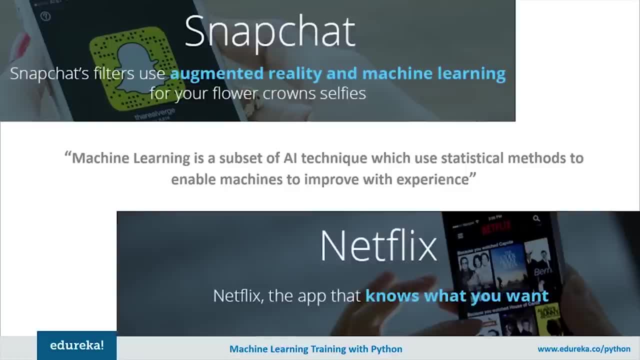 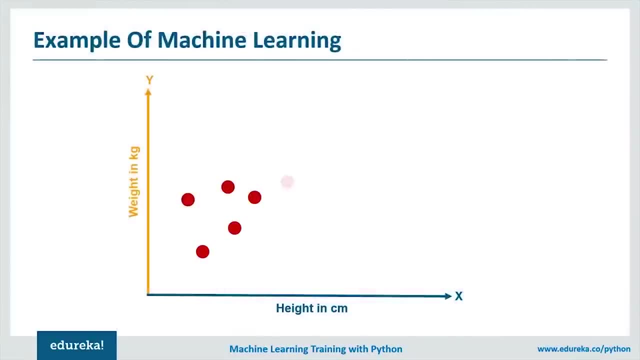 These programs or algorithms are designed in a way that they can learn and improve over time when exposed to new data. Let's see an example of machine learning. Let's say you want to create a system which tells the expected weight of a person based on its height. 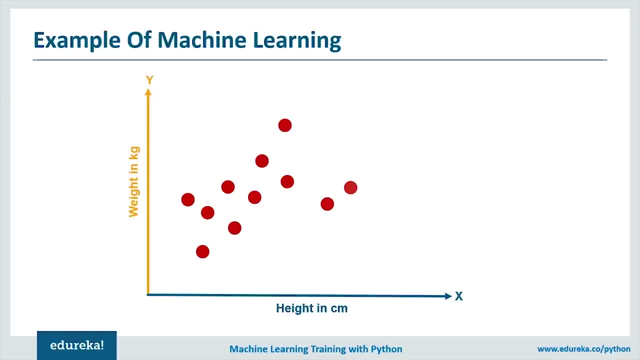 The first thing you do is you collect the data. Let's see. This is how your data looks like now. each point of the graph represent one data point. to start with, we can draw a simple line to predict the weight based on the height. For example, a simple line: W equal H minus 100. 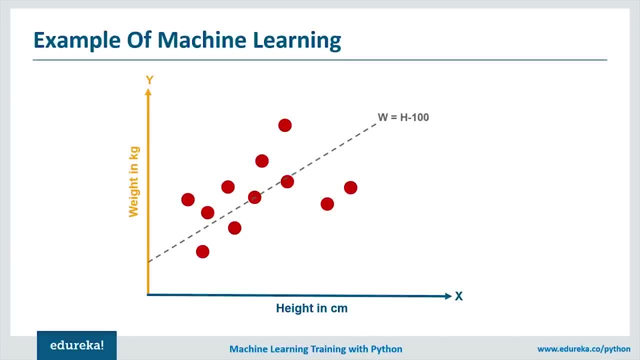 where W is weight in kgs and edges height in centimeter. This line can help us to make the prediction. Our main goal is to reduce the difference between the estimated value and the actual value, So in order to achieve it, we try to draw a straight line that fits. 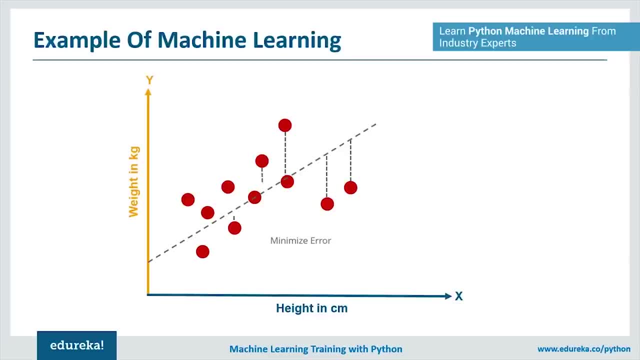 through all these different points and minimize the error. So our main goal is to minimize the error and make them as small as possible. decreasing the error or the difference between the actual value and estimated value increases the performance of the model further on the more data points. 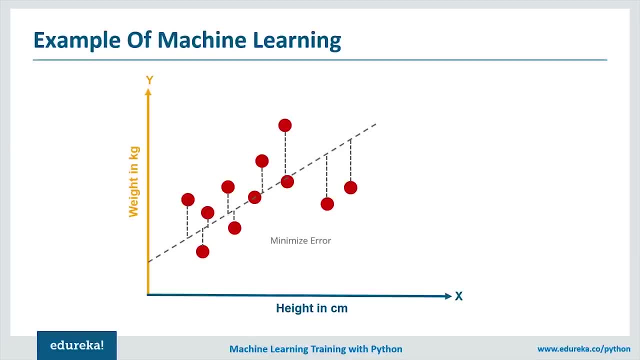 We collect, the better our model will become. we can also improve our model by adding more variables and creating different prediction lines for them Once the line is created. So from the next time, if we feed a new data, for example height of a person, to the model, 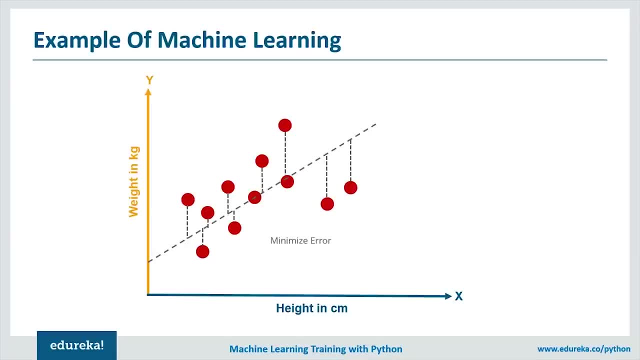 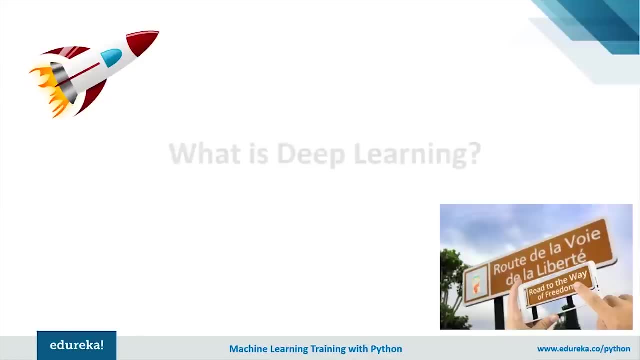 it would easily predict the data for you and it will tell you what is predicted weight could be. I hope you got a clear understanding of machine learning. So, moving on ahead, Let's learn about deep learning. Now, what is deep learning? You can consider deep learning model as a rocket engine. 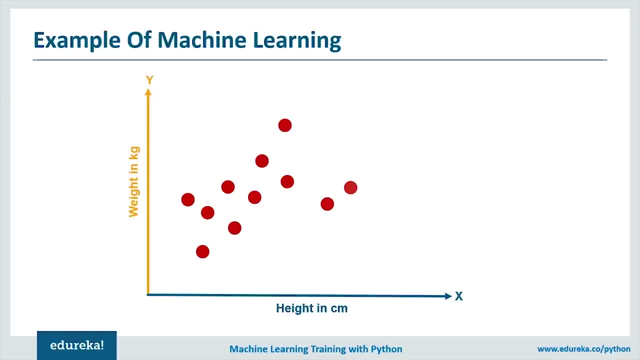 The first thing you do is you collect the data. Let's see. This is how your data looks like now. each point of the graph represent one data point. to start with, we can draw a simple line to predict the weight based on the height. For example, a simple line: W equal H minus 100. 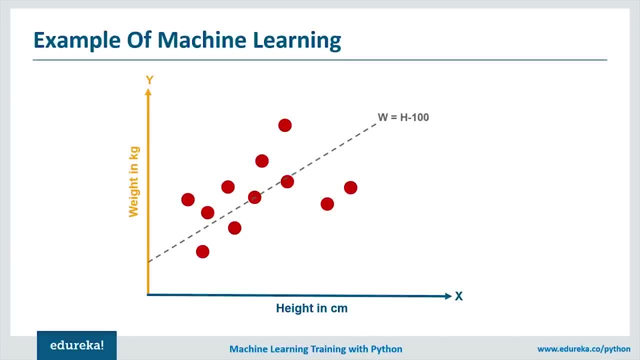 where W is weight in kgs and edges height in centimeter. This line can help us to make the prediction. Our main goal is to reduce the difference between the estimated value and the actual value, So in order to achieve it, we try to draw a straight line that fits. 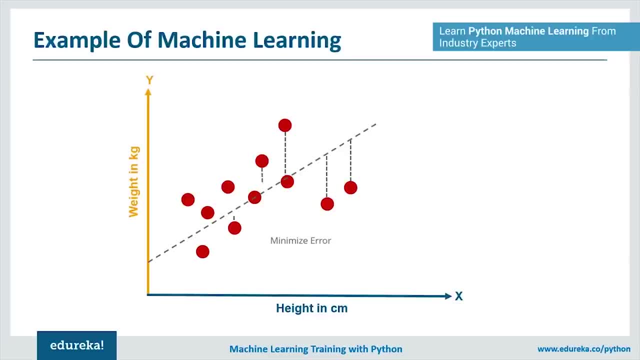 through all these different points and minimize the error. So our main goal is to minimize the error and make them as small as possible. decreasing the error or the difference between the actual value and estimated value increases the performance of the model further on the more data points. 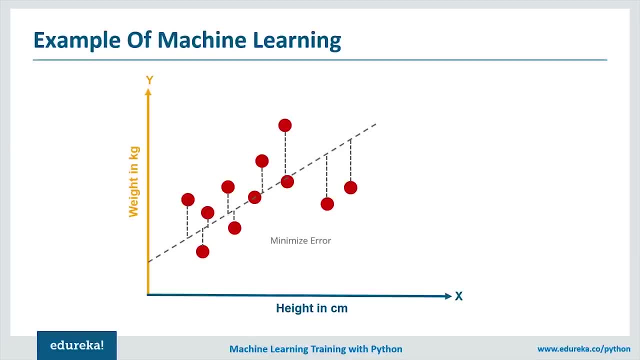 We collect, the better our model will become. we can also improve our model by adding more variables and creating different prediction lines for them Once the line is created. So from the next time, if we feed a new data, for example height of a person, to the model, 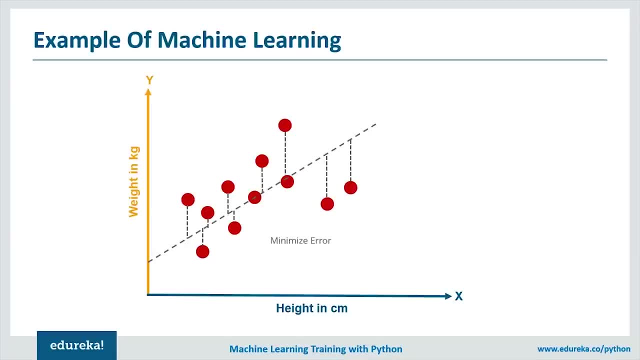 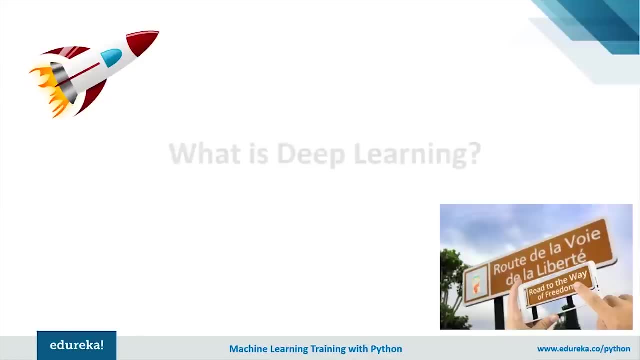 it would easily predict the data for you and it will tell you what is predicted weight could be. I hope you got a clear understanding of machine learning. So, moving on ahead, Let's learn about deep learning. Now, what is deep learning? You can consider deep learning model as a rocket engine. 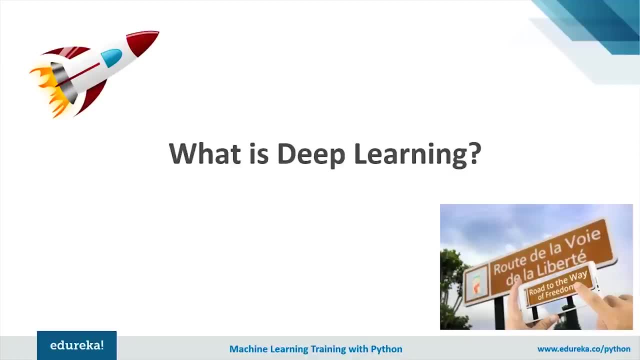 and its fuel is its huge amount of data that we feed to these algorithms. The concept of deep learning is not new, but recently its hype has increased and deep learning is getting more attention. This field, There's a particular kind of machine learning that is inspired by the functionality of our brain cells. 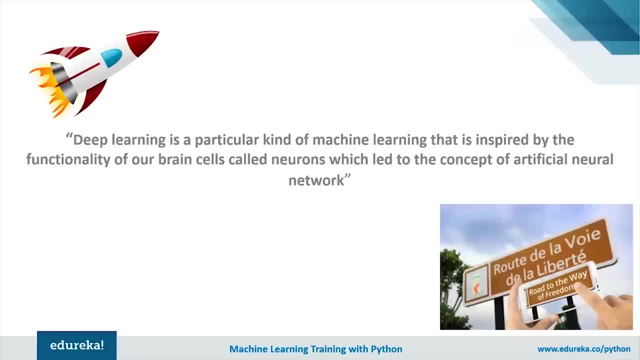 called neuron, which led to the concept of artificial neural network. It simply takes the data connection between all the artificial neurons and adjust them according to the data pattern. more neurons are added at the size of the data is large. It automatically features learning at multiple levels. 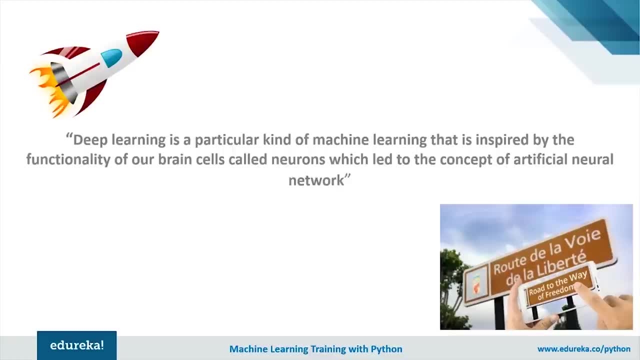 of abstraction, thereby allowing a system to learn complex function mapping without depending on any specific algorithm. You know what. No one actually knows what happens inside a neural network and why it works so well, So currently you can call it as a black box. Let us discuss some of the example of deep learning. 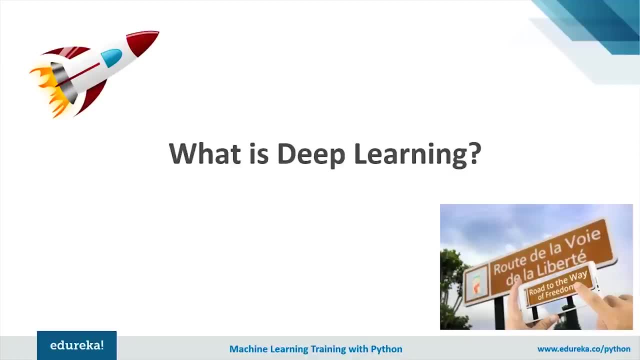 and its fuel is its huge amount of data that we feed to these algorithms. The concept of deep learning is not new, but recently its hype has increased and deep learning is getting more attention. This field, There's a particular kind of machine learning that is inspired by the functionality of our brain cells. 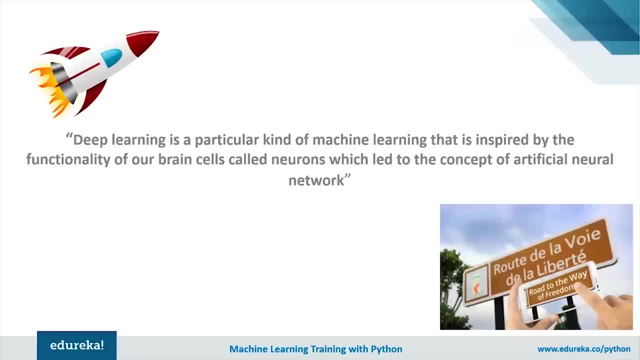 called neuron, which led to the concept of artificial neural network. It simply takes the data connection between all the artificial neurons and adjust them according to the data pattern. more neurons are added at the size of the data is large. It automatically features learning at multiple levels. 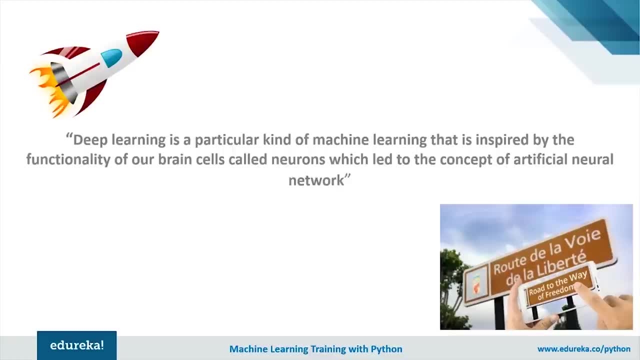 of abstraction, thereby allowing a system to learn complex function mapping without depending on any specific algorithm. You know what. No one actually knows what happens inside a neural network and why it works so well, So currently you can call it as a black box. Let us discuss some of the example of deep learning. 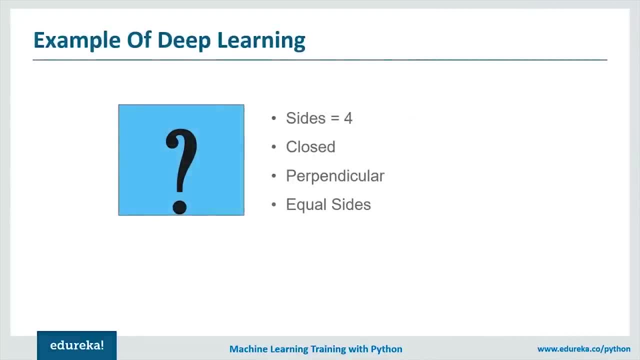 and understand it in a better way. Let me start with a simple example and explain you how things happen at a conceptual level. Let us try and understand how you recognize a square from other shapes. The first thing you do is you check whether there are four lines associated with the figure. 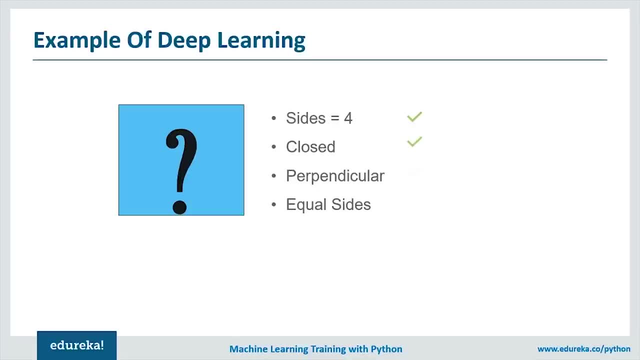 or not. simple concept, right? If yes, before the check if they are connected and closed again. if yes, we finally check whether it is perpendicular and all its sides are equal, correct? If everything fulfills, Yes, it is a square. 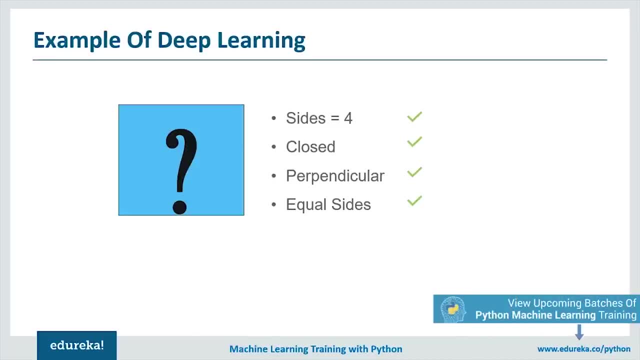 Well, it is nothing but a nested hierarchy of Concepts. What we did here? We took a complex task of identifying a square, in this case, and broke it into simpler task. Now this deep learning also does the same thing, but at a larger scale. 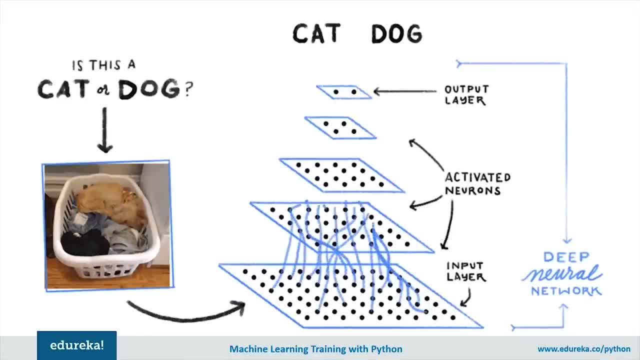 Let's take an example of machine which recognizes the animal. The task of the machine is to recognize whether the given image is of a cat or of a dog. What if we were asked to resolve the same issue using the concept of machine learning? what we would do first? 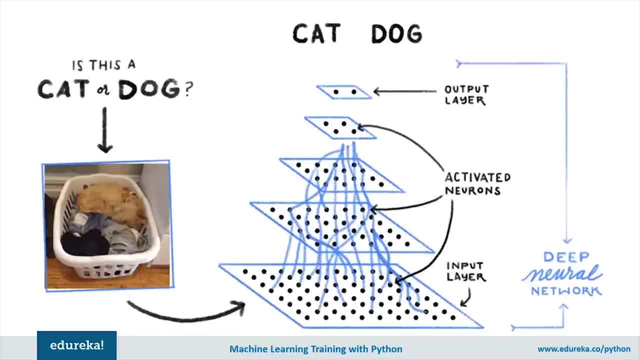 we would define the features, such as check whether the animal has whiskers or not, or check if the animal has pointed ears or not, or whether it's tail is straight or curved. in short, we will define the facial features and let the system identify which features are more important. 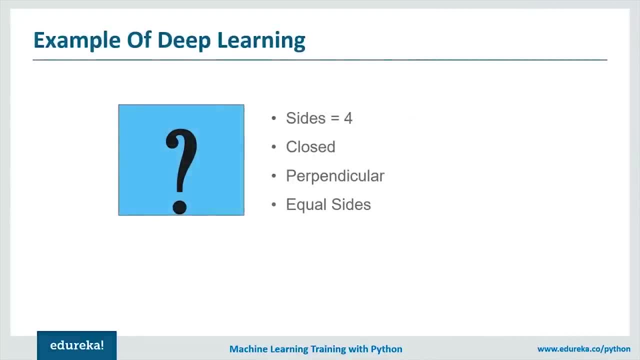 and understand it in a better way. Let me start with a simple example and explain you how things happen at a conceptual level. Let us try and understand how you recognize a square from other shapes. The first thing you do is you check whether there are four lines associated with the figure. 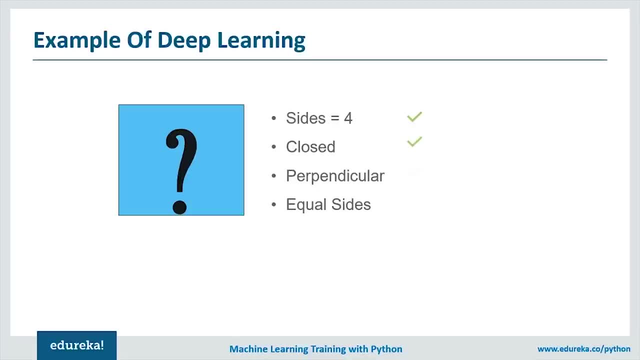 or not. simple concept, right? If yes, before the check if they are connected and closed again. if yes, we finally check whether it is perpendicular and all its sides are equal, correct? If everything fulfills, Yes, it is a square. 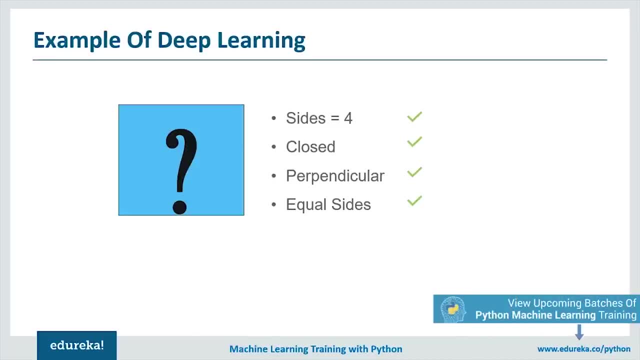 Well, it is nothing but a nested hierarchy of Concepts. What we did here? We took a complex task of identifying a square, in this case, and broke it into simpler task. Now this deep learning also does the same thing, but at a larger scale. 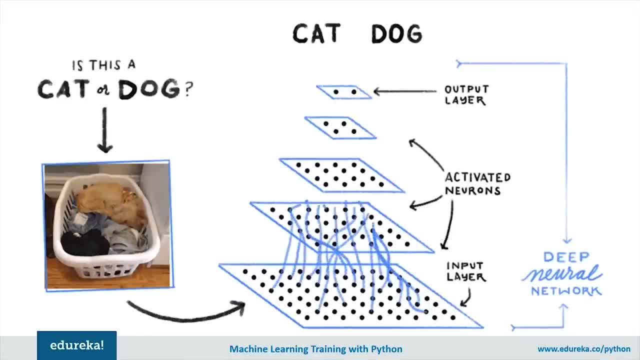 Let's take an example of machine which recognizes the animal. The task of the machine is to recognize whether the given image is of a cat or of a dog. What if we were asked to resolve the same issue using the concept of machine learning? what we would do first? 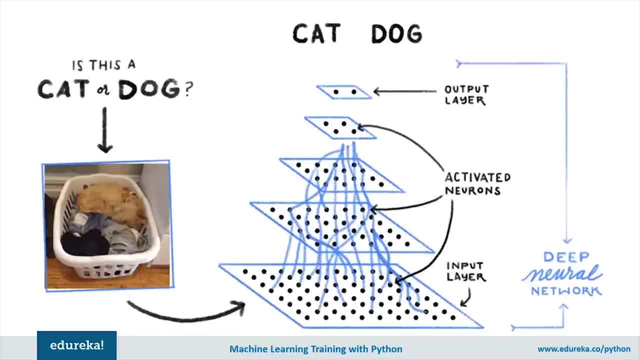 we would define the features, such as check whether the animal has whiskers or not, or check if the animal has pointed ears or not, or whether it's tail is straight or curved. in short, we will define the facial features and let the system identify which features are more important. 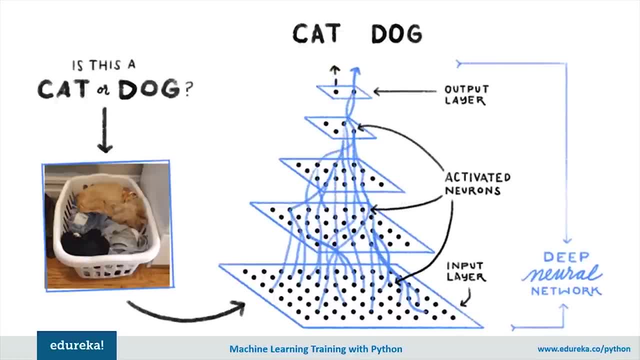 in classifying a particular animal. Now, when it comes to deep learning, it takes this to one step ahead. deep learning automatically finds out the feature which are most important for classification, compared to machine learning where we had to manually give out that features. by now I guess you have understood that AI is a bigger picture. 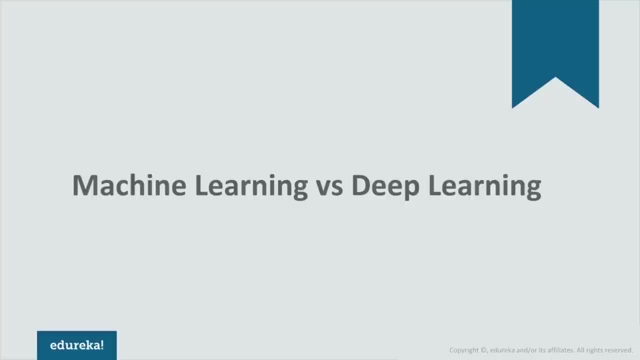 and machine learning and deep learning are its subpart. So let's move on and focus our discussion on machine learning and deep learning. the easiest way to understand the difference between the machine learning and deep learning is to know that deep learning is machine learning. more specifically, 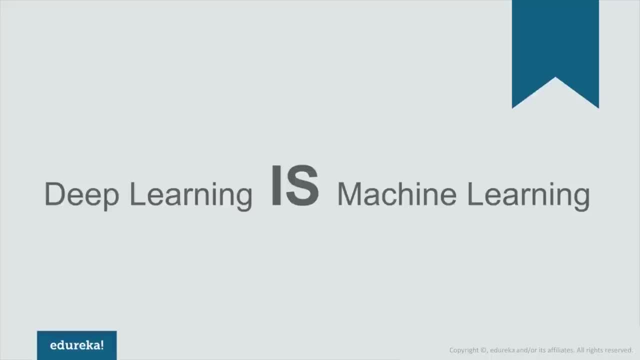 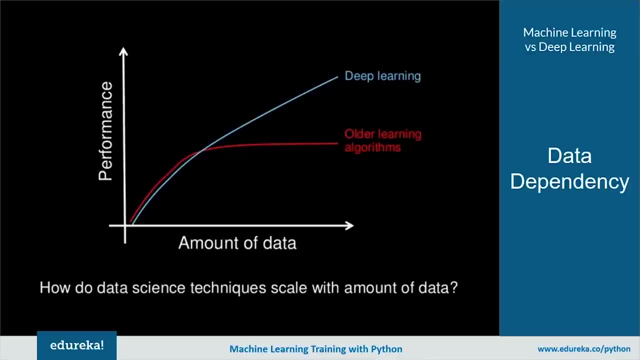 It is the next evolution of machine learning. Let's take few important parameter and compare machine learning with deep learning. So, starting with data dependencies, the most important difference between deep learning and machine learning is its performance as the volume of the data gets increased. from the below graph, 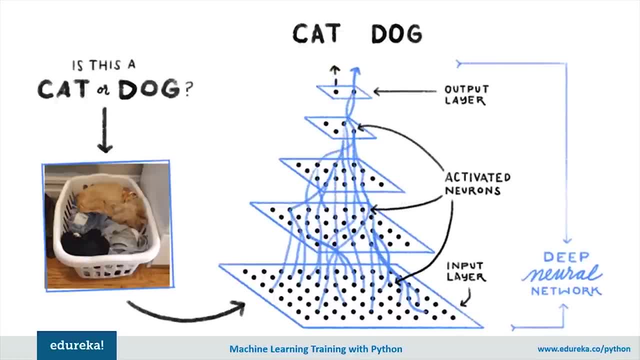 in classifying a particular animal. Now, when it comes to deep learning, it takes this to one step ahead. deep learning automatically finds out the feature which are most important for classification, compared to machine learning where we had to manually give out that features. by now I guess you have understood that AI is a bigger picture. 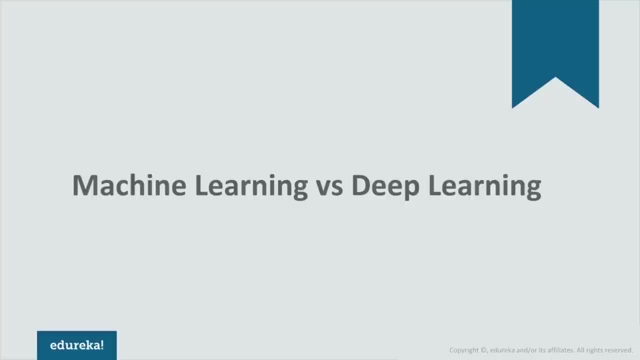 and machine learning and deep learning are its subpart. So let's move on and focus our discussion on machine learning and deep learning. the easiest way to understand the difference between the machine learning and deep learning is to know that deep learning is machine learning. more specifically, 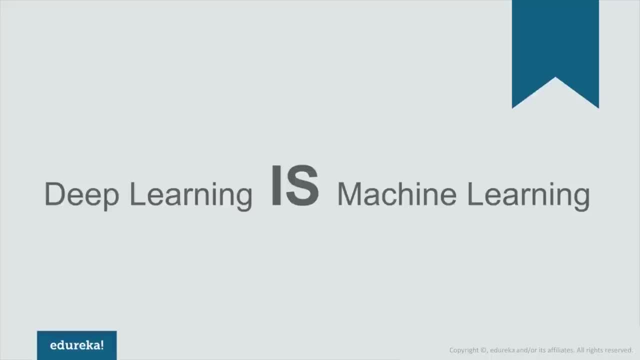 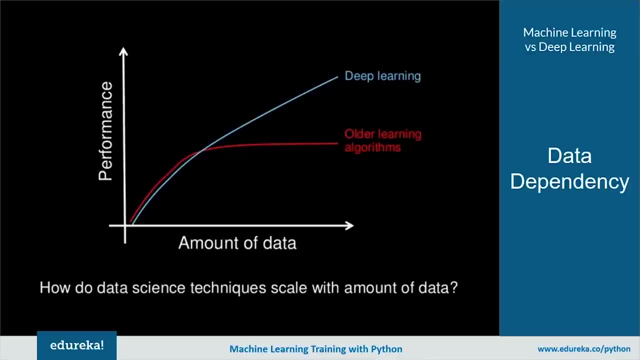 It is the next evolution of machine learning. Let's take few important parameter and compare machine learning with deep learning. So, starting with data dependencies, the most important difference between deep learning and machine learning is its performance as the volume of the data gets increased. from the below graph, 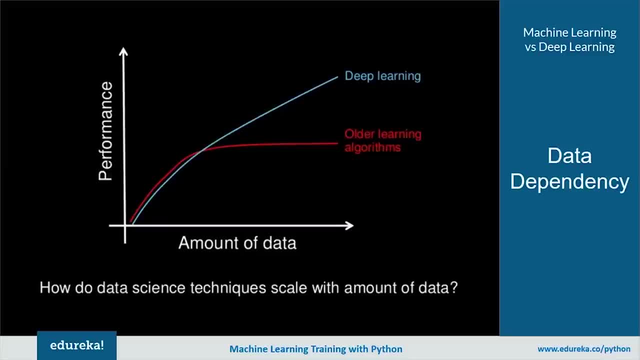 You can see that when the size of the data is small, deep learning algorithm doesn't perform that well. but why? well, this is because deep learning algorithm needs a large amount of data to understand it perfectly. on the other hand, the machine learning algorithm can easily work. 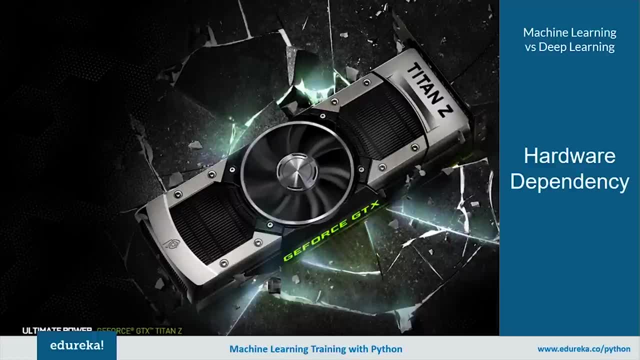 with smaller data set fine. next comes the hardware dependencies. deep learning algorithms are heavily dependent on high-end machines, while the machine learning algorithm can work on low-end machines as well. This is because the requirement of deep learning algorithm include GPUs, which is an integral part of its working. the deep learning 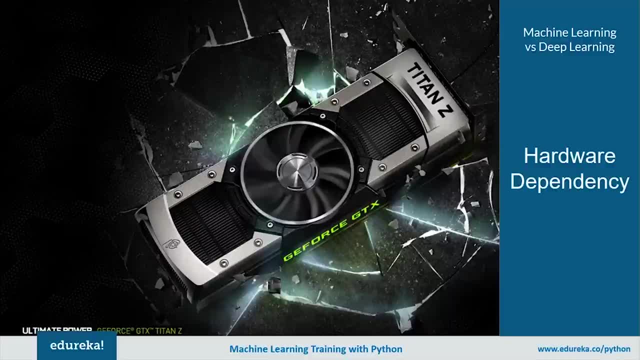 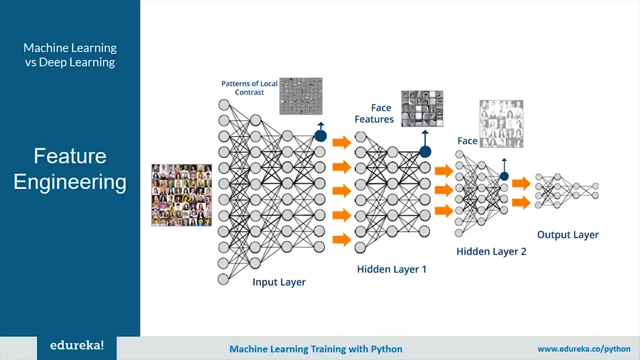 algorithm required GPUs, as they do a large amount of matrix multiplication operations, And these operations can only be efficiently optimized using a GPU as it is built for this purpose only. our third parameter will be feature engineering. Well, feature engineering is a process of putting the domain knowledge to reduce the complexity. 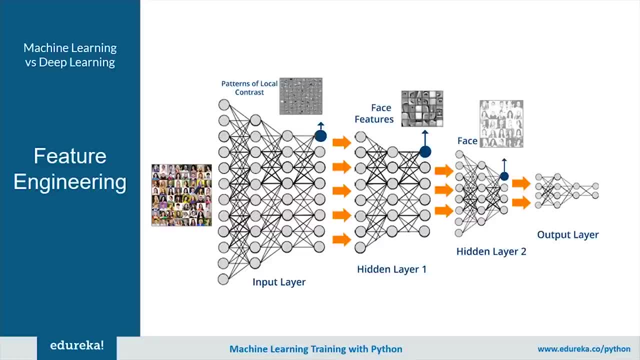 of the data and make patterns more visible to learning algorithms. This process is difficult and expensive in terms of time and expertise. in case of machine learning, most of the features are needed to be identified by an expert and then hand-coded as per the domain and the data type. for example, 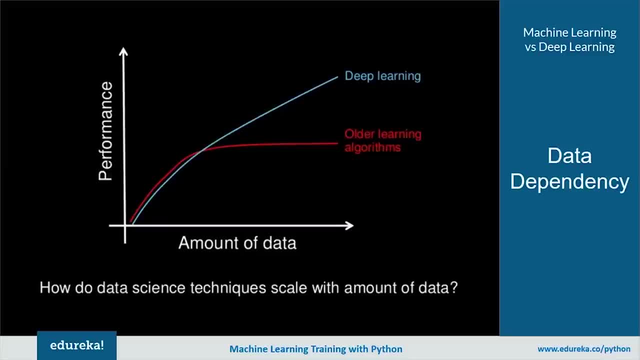 You can see that when the size of the data is small, deep learning algorithm doesn't perform that well. but why? well, this is because deep learning algorithm needs a large amount of data to understand it perfectly. on the other hand, the machine learning algorithm can easily work. 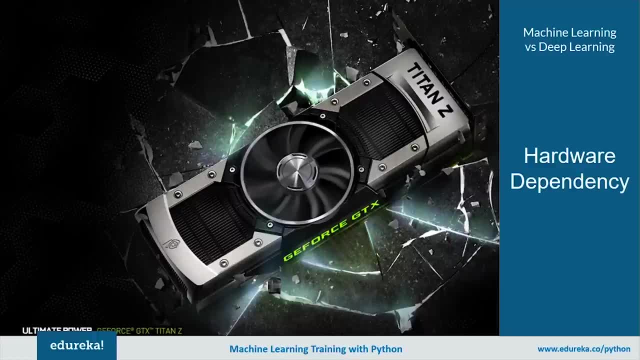 with smaller data set fine. next comes the hardware dependencies. deep learning algorithms are heavily dependent on high-end machines, while the machine learning algorithm can work on low-end machines as well. This is because the requirement of deep learning algorithm include GPUs, which is an integral part of its working. the deep learning 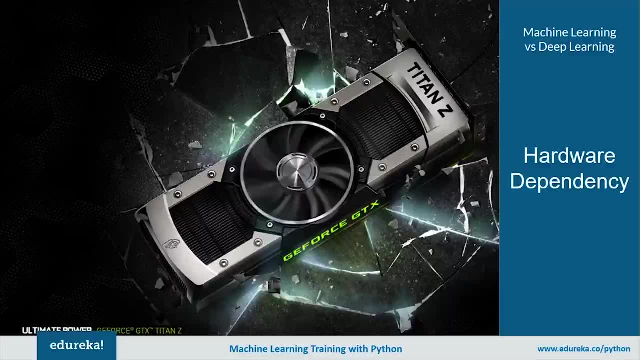 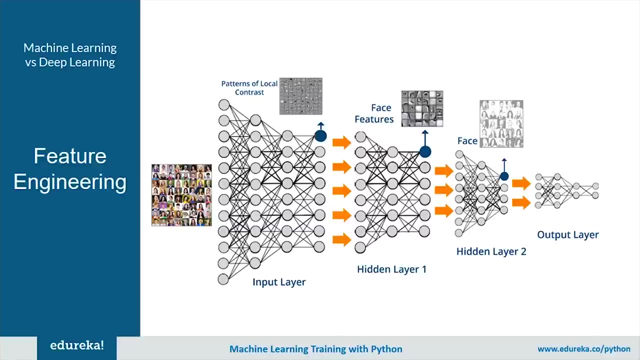 algorithm required GPUs, as they do a large amount of matrix multiplication operations, And these operations can only be efficiently optimized using a GPU as it is built for this purpose only. our third parameter will be feature engineering. Well, feature engineering is a process of putting the domain knowledge to reduce the complexity. 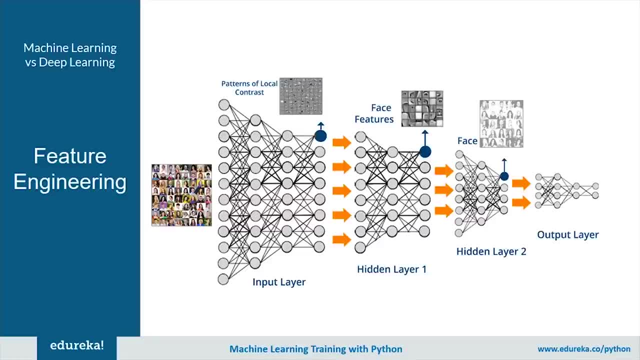 of the data and make patterns more visible to learning algorithms. This process is difficult and expensive in terms of time and expertise. in case of machine learning, most of the features are needed to be identified by an expert and then hand-coded as per the domain and the data type. for example, 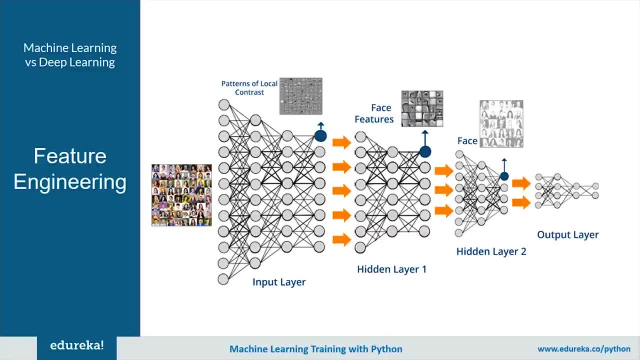 the features can be a pixel value, shapes, texture, position, orientation or anything fine. the performance of most of the machine learning algorithm depends on how accurately the features are identified and extracted, whereas in case of deep learning algorithms it try to learn high-level features from the data. 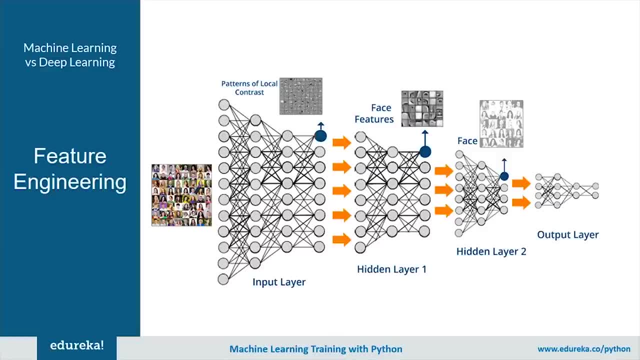 This is a very distinctive part of deep learning which makes it way ahead of traditional machine learning. deep learning reduces. It is a task of developing new feature extractor for every problem. like in the case of CNN algorithm, It first try to learn the low-level features. 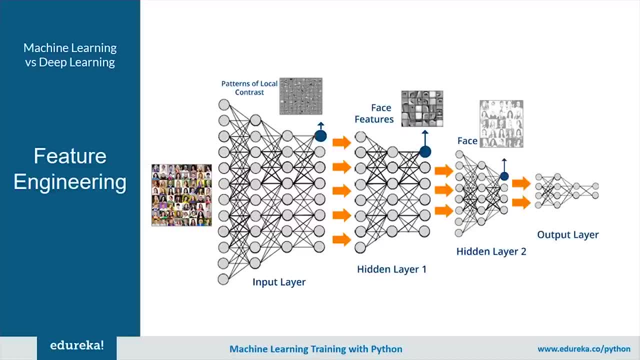 of the image, such as edges and lines, and then it proceeds to the parts of faces of people and then, finally, to the high-level representation of the face. I hope the things are getting clear to you, So let's move on ahead and see the next parameter. 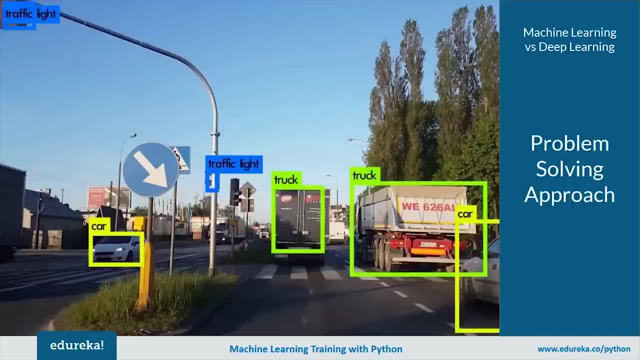 So our next parameter is problem-solving approach. when we are solving a problem using traditional machine learning algorithm, It is generally recommended that we first break down the problem into different subparts, solve them individually and then finally combine them to get the desired result. This is how the machine learning algorithm handles the problem. 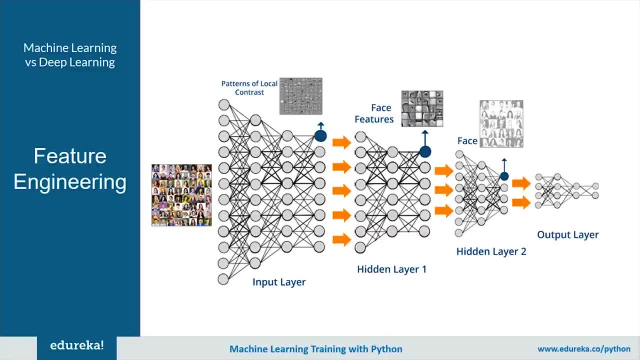 the features can be a pixel value, shapes, texture, position, orientation or anything fine. the performance of most of the machine learning algorithm depends on how accurately the features are identified and extracted, whereas in case of deep learning algorithms it try to learn high-level features from the data. 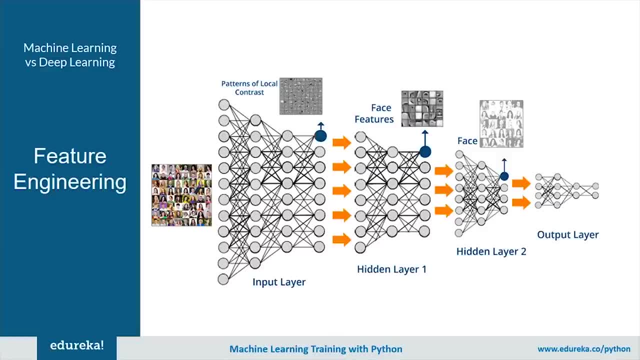 This is a very distinctive part of deep learning which makes it way ahead of traditional machine learning. deep learning reduces. It is a task of developing new feature extractor for every problem. like in the case of CNN algorithm, It first try to learn the low-level features. 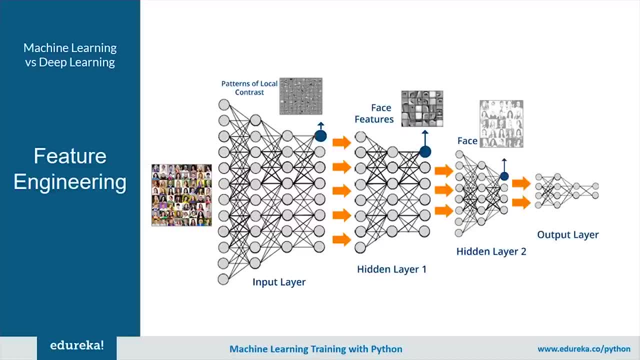 of the image, such as edges and lines, and then it proceeds to the parts of faces of people and then, finally, to the high-level representation of the face. I hope the things are getting clear to you, So let's move on ahead and see the next parameter. 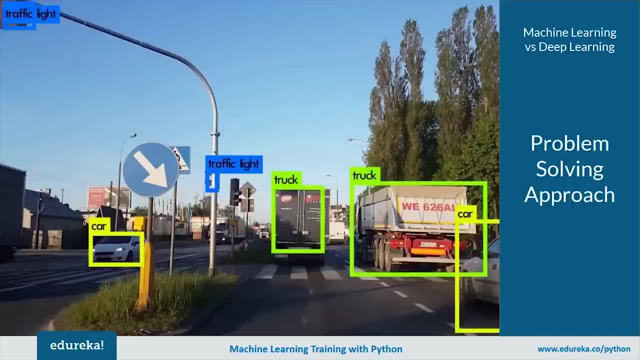 So our next parameter is problem-solving approach. when we are solving a problem using traditional machine learning algorithm, It is generally recommended that we first break down the problem into different subparts, solve them individually and then finally combine them to get the desired result. This is how the machine learning algorithm handles the problem. 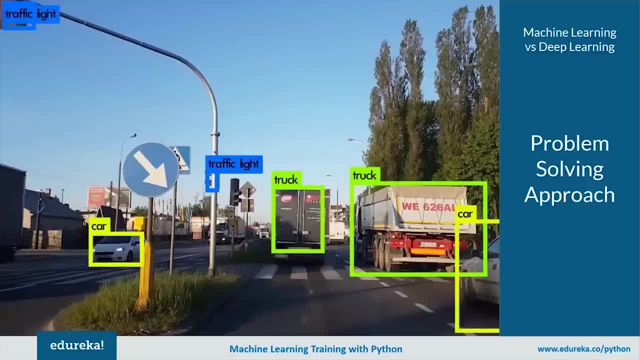 On the other hand, the deep learning algorithm solves the problem from end to end. Let's take an example to understand this. suppose you have a task of multiple object detection and your task is to identify what is the object and where it is present in the image. 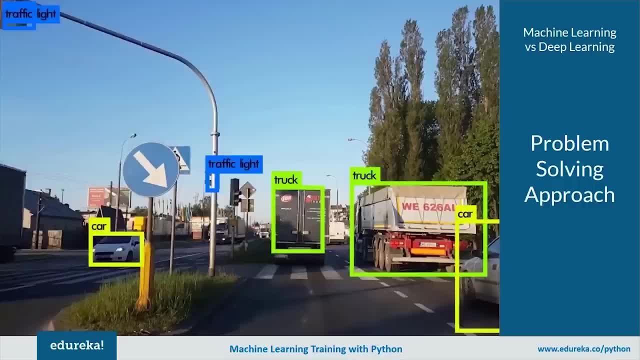 So let's see and compare. how will you tackle this issue using the concept of machine learning and deep learning, starting with machine learning. in a typical machine learning approach, You would first divide the problem into two step: first object detection and then object organization. First of all, you would use a bounding box detection algorithm. 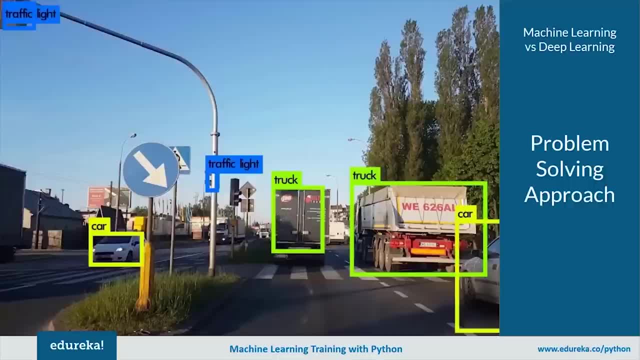 like grab-cut, for example, to scan through the image and find out all the possible objects. Now, once the objects are recognized, you would use object organization algorithm like SVM with hog to recognize relevant objects. Now, finally, when you combine the result, you would be able to identify what is the object. 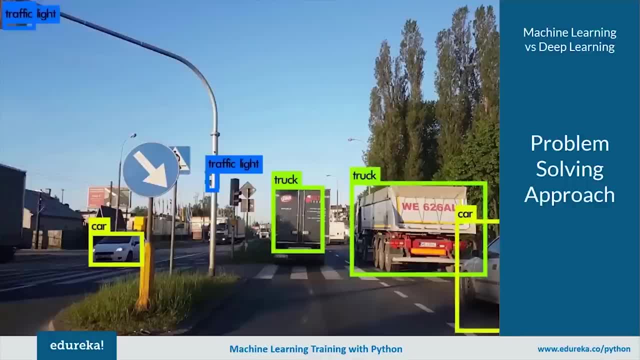 and where it is present in the image. on the other hand, and deep learning approach: you would do the process from end to end. for example, in a Yolo net, which is a type of deep learning algorithm. you would pass an image and it would give out the location along. 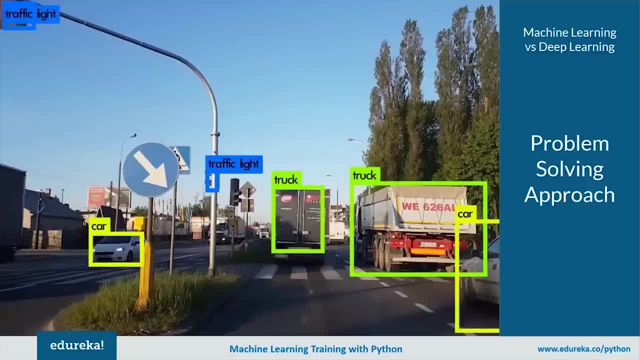 On the other hand, the deep learning algorithm solves the problem from end to end. Let's take an example to understand this. suppose you have a task of multiple object detection and your task is to identify what is the object and where it is present in the image. 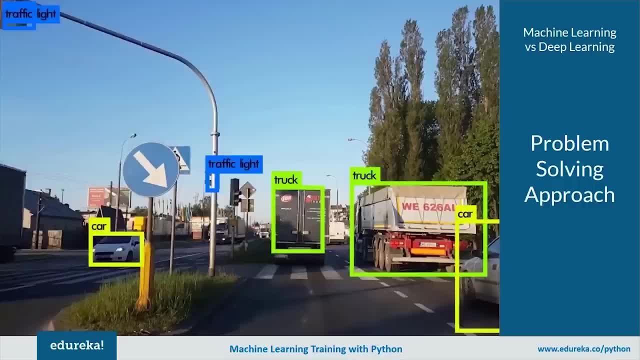 So let's see and compare. how will you tackle this issue using the concept of machine learning and deep learning, starting with machine learning. in a typical machine learning approach, You would first divide the problem into two step: first object detection and then object organization. First of all, you would use a bounding box detection algorithm. 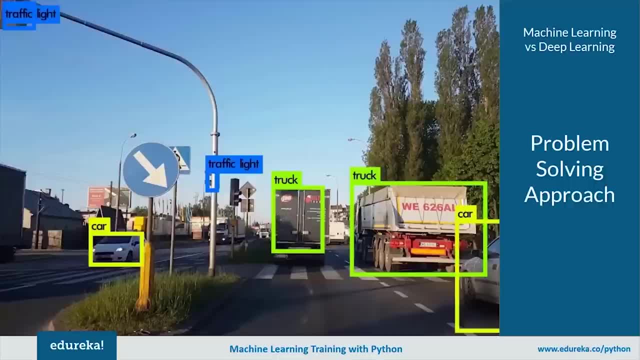 like grab-cut, for example, to scan through the image and find out all the possible objects. Now, once the objects are recognized, you would use object organization algorithm like SVM with hog to recognize relevant objects. Now, finally, when you combine the result, you would be able to identify what is the object. 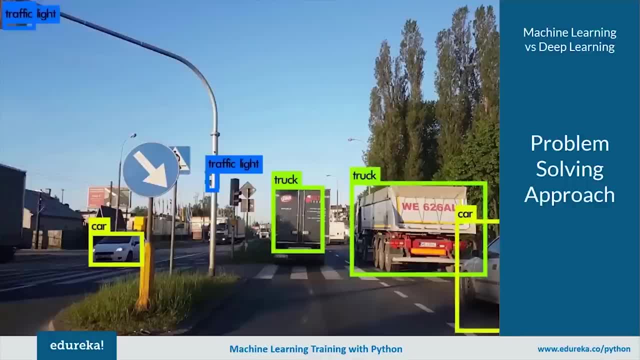 and where it is present in the image. on the other hand, and deep learning approach: you would do the process from end to end. for example, in a Yolo net, which is a type of deep learning algorithm. you would pass an image and it would give out the location along. 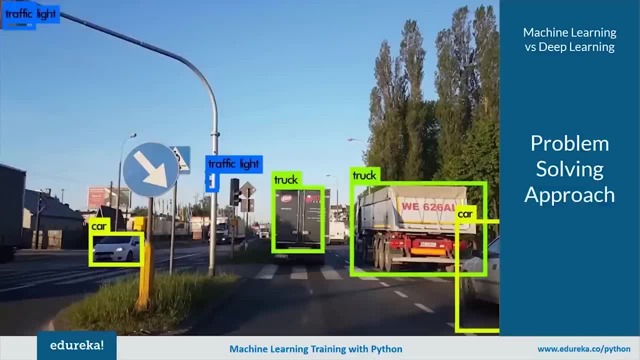 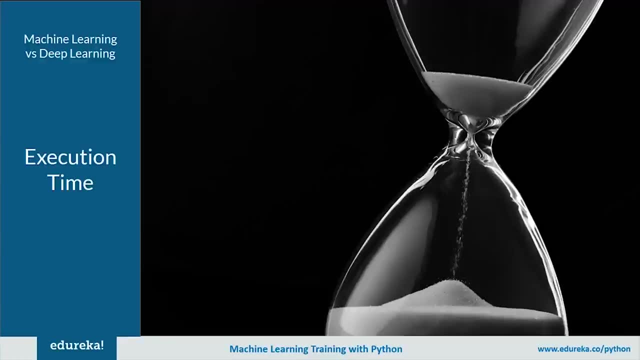 with the name of the object. Now let's move on to our fifth comparison parameter. It's execution time. usually, a deep learning algorithm takes a long time to train this. because there's so many parameter in a deep learning algorithm, that makes the training longer. 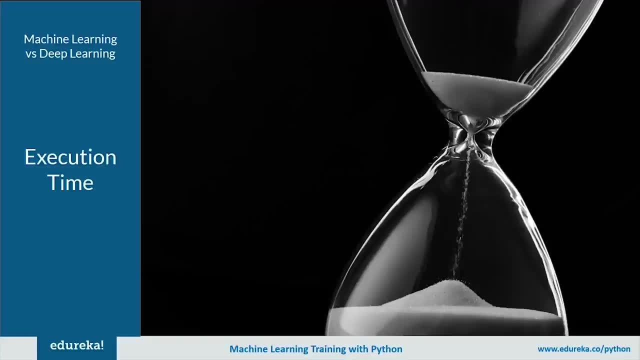 than usual. the training might even last for two weeks, or more than that if you are training completely from the scratch, whereas in the case of machine learning, it relatively takes much less time to train, ranging from a few weeks to few hours. Now the execution time is completely reverse. 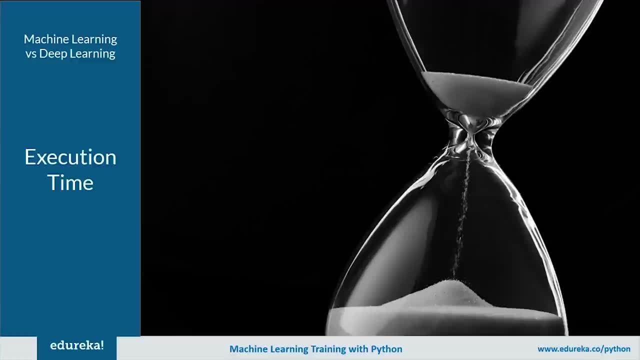 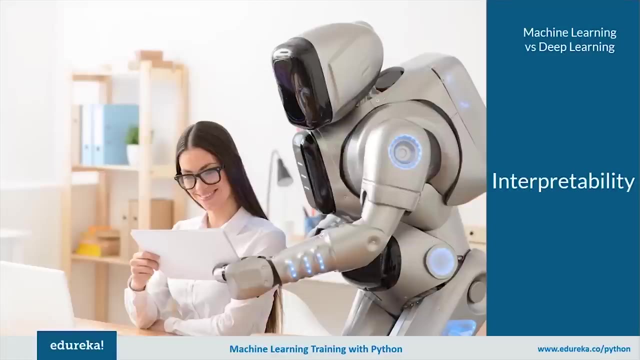 when it comes to the testing of data during testing, the deep learning algorithm takes much less time to run, whereas if you compare it with a cannon algorithm, which is a type of machine learning algorithm, the test time increases as the size of the data increase. last but not the least, we have interpretability as a factor. 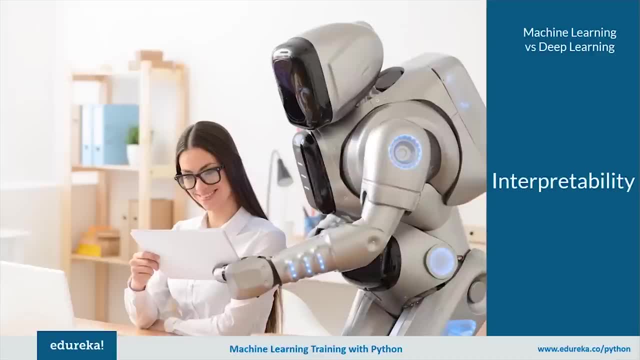 for comparison of machine learning and deep learning. This factor is the main reason why deep learning is still taught 10 times before anyone uses it in the industry. Let's take an example. Suppose we use deep learning to give automated scoring to essays. the performance it gives in scoring is quite excellent. 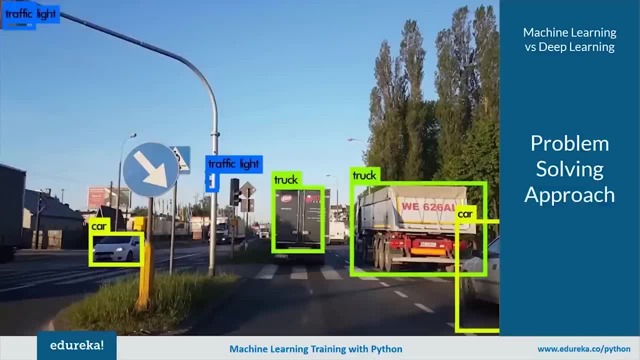 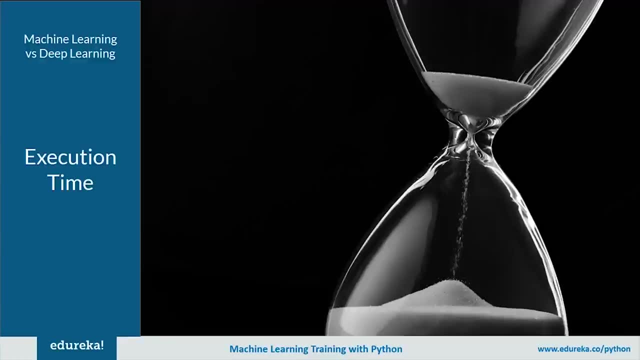 with the name of the object. Now let's move on to our fifth comparison parameter. It's execution time. usually, a deep learning algorithm takes a long time to train this. because there's so many parameter in a deep learning algorithm, that makes the training longer. 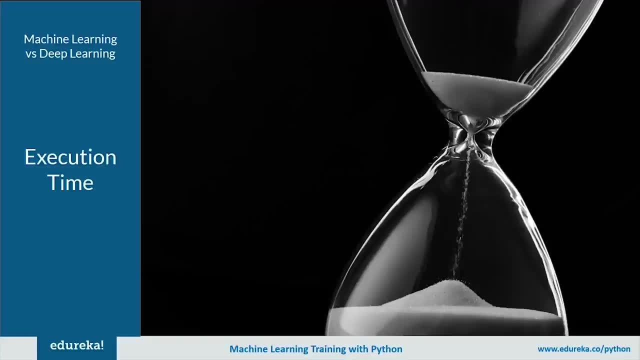 than usual. the training might even last for two weeks, or more than that if you are training completely from the scratch, whereas in the case of machine learning, it relatively takes much less time to train, ranging from a few weeks to few hours. Now the execution time is completely reverse. 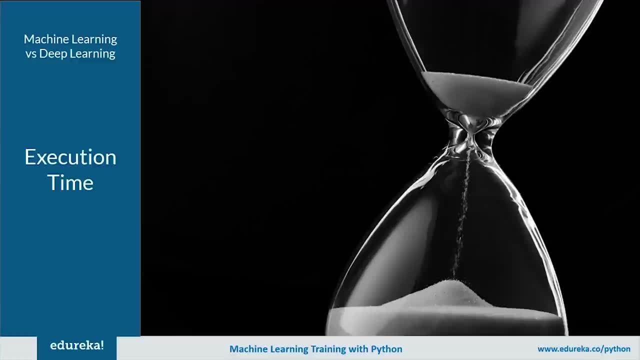 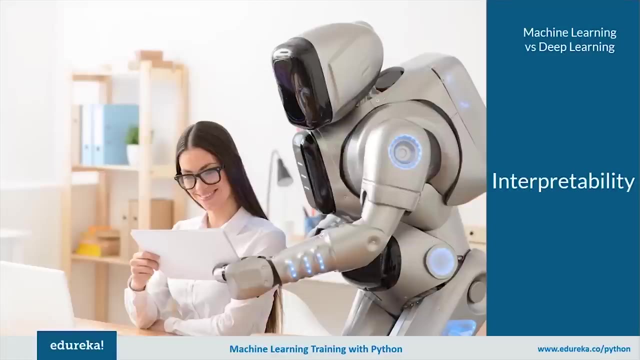 when it comes to the testing of data during testing, the deep learning algorithm takes much less time to run, whereas if you compare it with a cannon algorithm, which is a type of machine learning algorithm, the test time increases as the size of the data increase. last but not the least, we have interpretability as a factor. 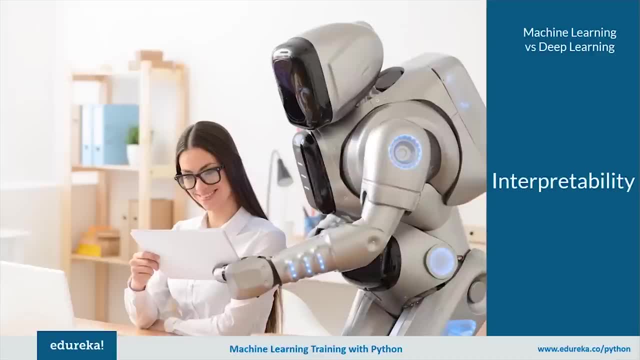 for comparison of machine learning and deep learning. This factor is the main reason why deep learning is still taught 10 times before anyone uses it in the industry. Let's take an example. Suppose we use deep learning to give automated scoring to essays. the performance it gives in scoring is quite excellent. 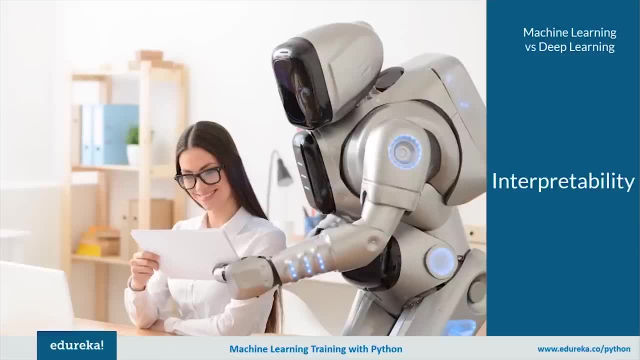 and is near to the human Performance. but there's an issue with it: It does not reveal why it has given that score. Indeed, mathematically it is possible to find out that which node of a deep neural network were activated, but we don't know what the neurons are supposed to model. 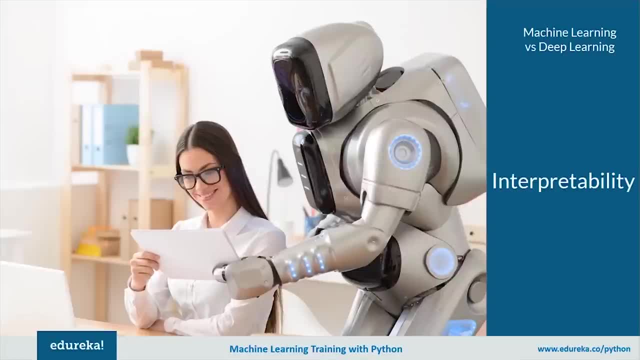 and what these layers of neuron were doing collectively, So he failed to interpret the result. on the other hand, machine learning algorithm, like decision tree, gives us a crisp rule for why it chose and what it chose, So it is particularly easy to interpret the reasoning behind. 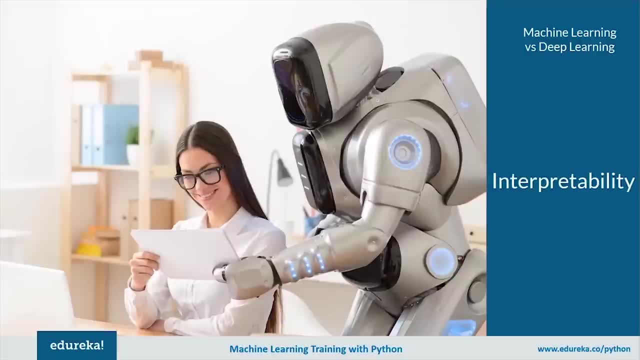 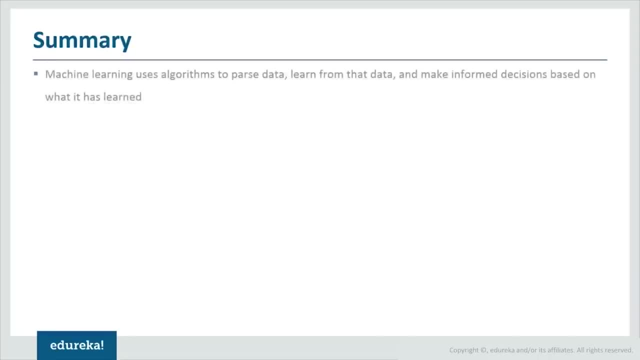 it. Therefore, the algorithms like decision tree and linear or logistic regression are primarily used in industry for interpret ability. Let me summarize things for you. machine learning uses algorithm to parse the data, learn from the data and make informed decision based on what it has learned. fine, 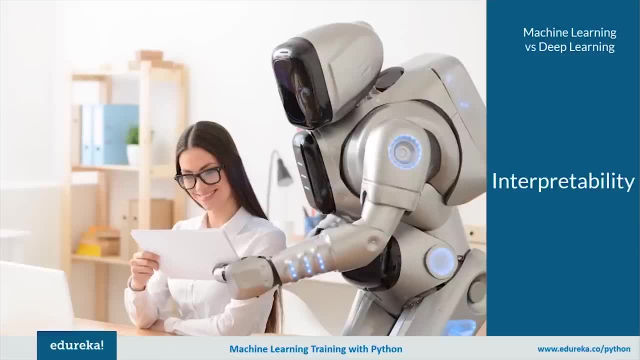 and is near to the human Performance. but there's an issue with it: It does not reveal why it has given that score. indeed, mathematically it is possible to find out that which node of a deep neural network were activated, but we don't know what the neurons are supposed to model. 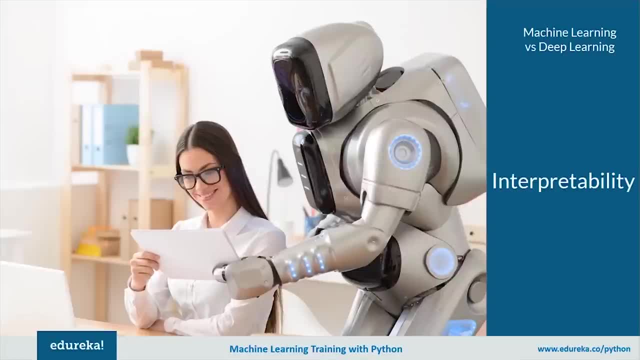 and what these layers of neuron were doing collectively, So he failed to interpret the result. on the other hand, machine learning algorithm, like decision tree, gives us a crisp rule for why it chose and what it chose, So it is particularly easy to interpret the reasoning behind. 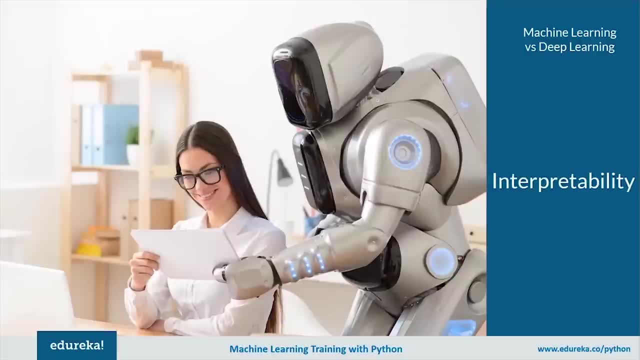 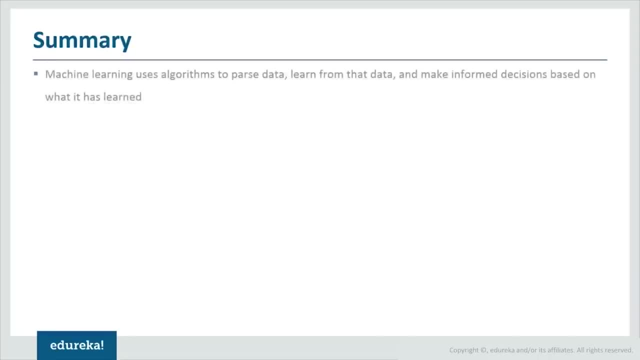 it. Therefore, the algorithms like decision tree and linear or logistic regression are primarily used in industry for interpret ability. Let me summarize things for you. machine learning uses algorithm to parse the data, learn from the data and make informed decision based on what it has learned. fine, 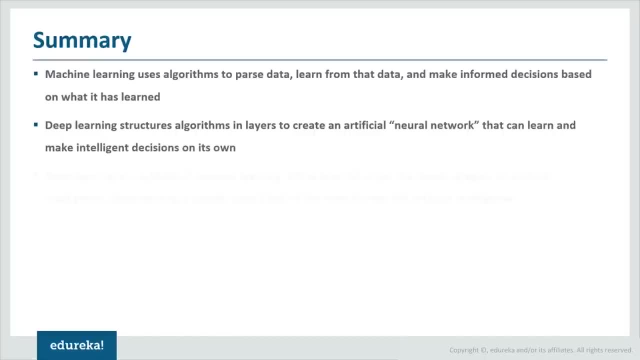 Now this deep learning structures algorithms and layers to create artificial neural network that can learn and make intelligent decisions on their own. finally, deep learning is a subfield of machine learning, while both fall under the broad category of artificial intelligence. deep learning is usually what's behind, the most human, like artificial intelligence. 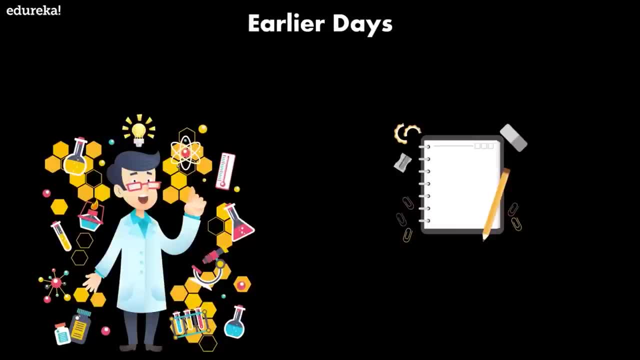 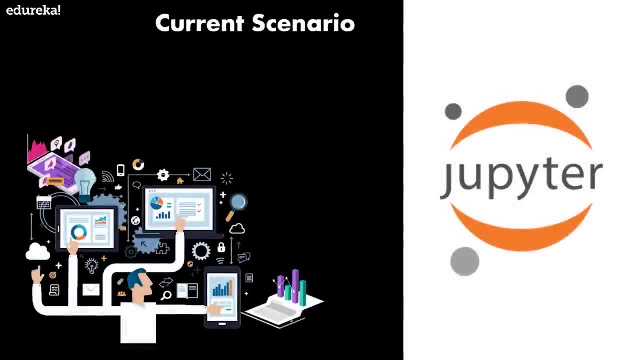 Now, in early days, scientists used to have a lab notebook to record tests, progress results and conclusions. Now Jupiter is a modern-day tool that allows data scientists to record their complete analysis process much in the same way Other scientists use a lab notebook. now the Jupiter product. 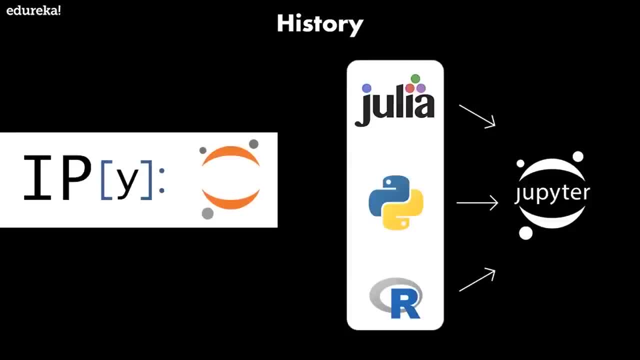 was originally developed as a part of ipython project. The ipython project was used to provide interactive online access to python. over time, It became useful to interact with other data analysis tools such as are: in the same manner, with the split from python, the tool grew into its current manifestation of Jupiter. 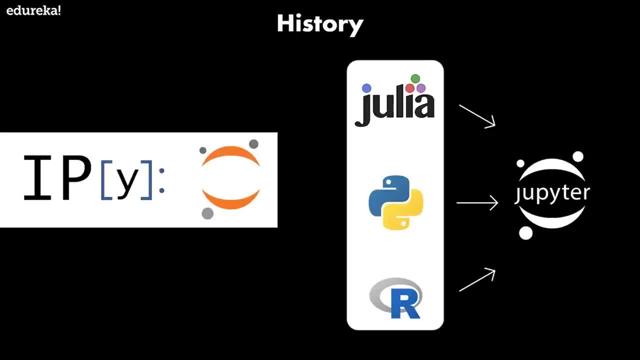 Now ipython is still an active tool that's available for use. the name Jupiter itself is derived from the combination of Julia, Python and are. while Jupiter runs code in many programming languages. python is a requirement for installing the Jupiter notebook itself, not to download Jupiter notebook. 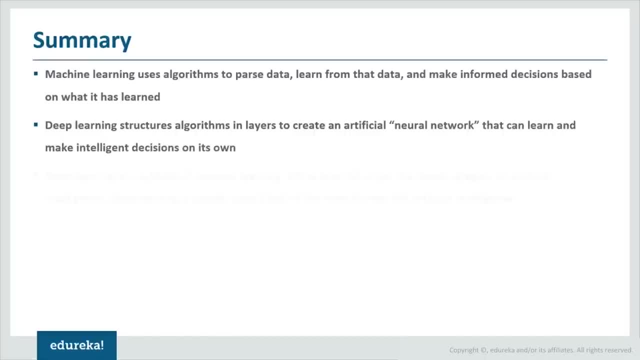 Now this deep learning structures algorithms and layers to create artificial neural network that can learn and make intelligent decisions on their own. finally, deep learning is a subfield of machine learning, while both fall under the broad category of artificial intelligence. deep learning is usually what's behind, the most human, like artificial intelligence. 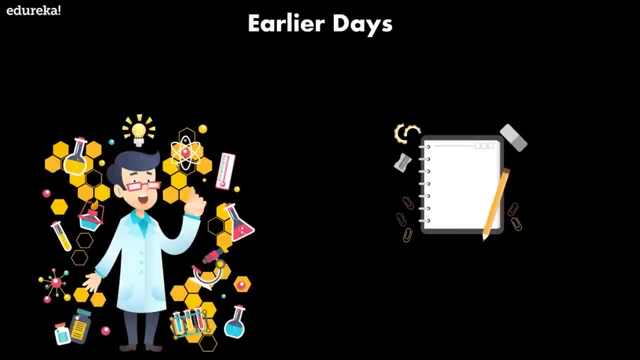 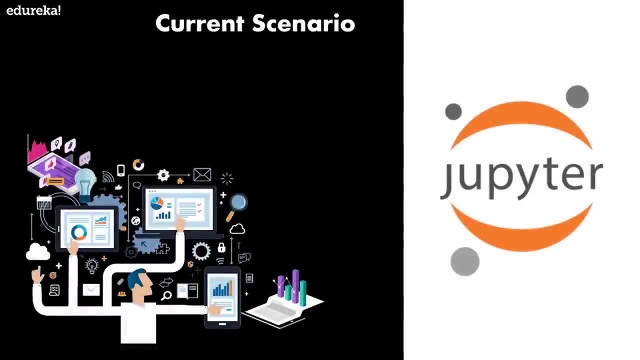 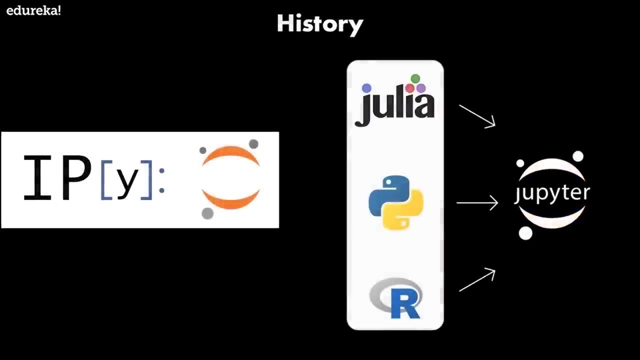 Now. in early days, scientists used to have a lab notebook to record tests, progress results and conclusions. now, Jupiter is a modern-day tool that allows data scientists to record their complete analysis process, much in the same way other scientists use a lab notebook Now. the Jupiter product was originally developed as a part 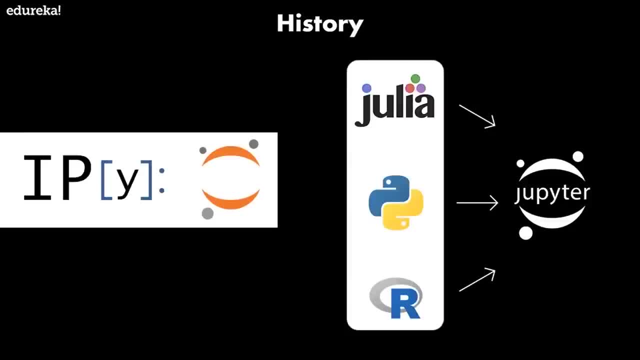 of ipython project. the ipython project was used to provide interactive online access to python. over time, it became useful to interact with other data analysis tools such as are: in the same manner, with the split from python, the tool grew into its current manifestation of Jupiter. 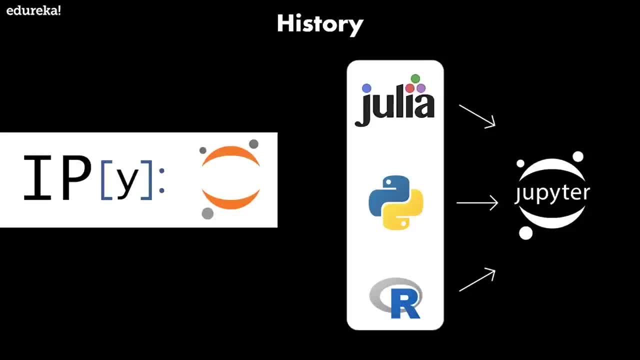 Now ipython is still an active tool that's available for use. the name Jupiter itself is derived from the combination of Julia, Python and are. while Jupiter runs code in many programming languages. python is a requirement for installing the Jupiter notebook itself, not to download Jupiter notebook. 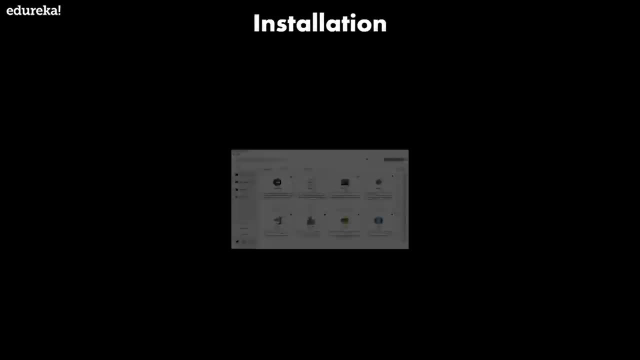 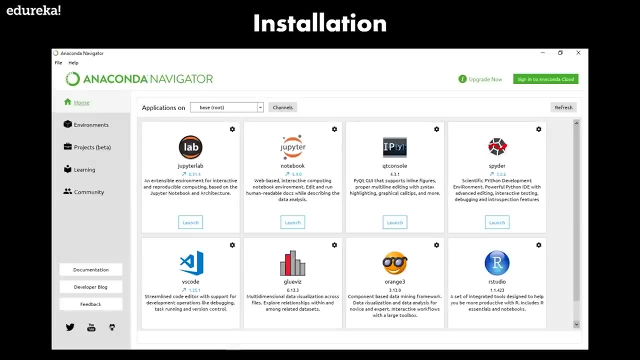 There are a few ways in their official website. It is strongly recommended installing python and Jupiter using anaconda distribution, which includes python, the Jupiter notebook and other commonly used packages for scientific computing as well as data science, Although one can also do so using the pip installation method. 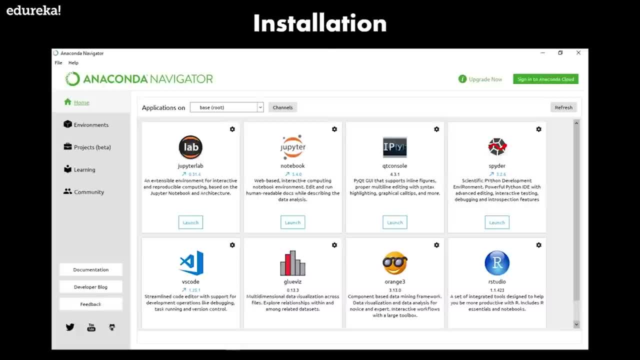 personally, What I would suggest is downloading anaconda navigator, which is a desktop graphical user interface included in anaconda Now. this allows you to launch application and easily manage conda packages, environments and channels without the need to use command line commands. So all you need to do is go to anacondaorg and inside you go. 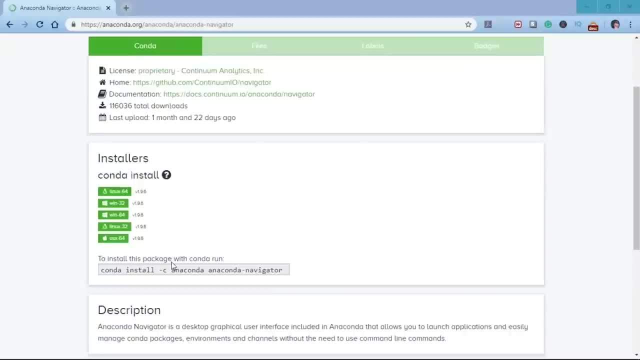 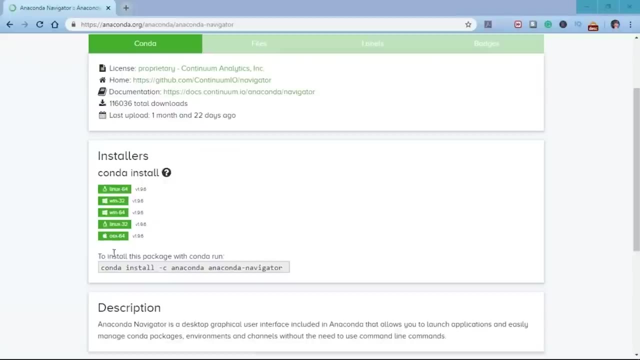 to anaconda navigator. So, as you can see, here we have the conda installation code which you're going to use to install it in your particular PC. So either you can Use these installers, So once you download the anaconda navigator it looks something. 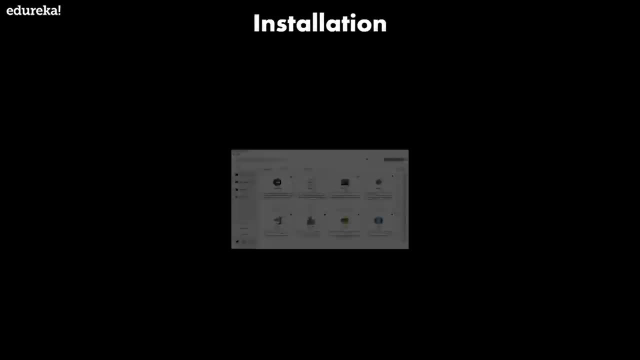 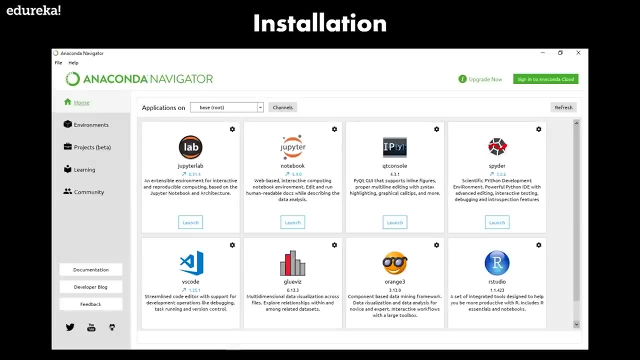 There are a few ways in their official website. It is strongly recommended installing python and Jupiter using anaconda distribution, which includes python, the Jupiter notebook and other commonly used packages for scientific computing as well as data science, Although one can also do so using the pip installation method. 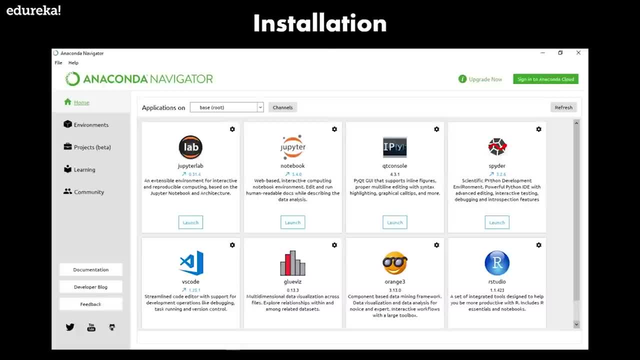 personally, What I would suggest is downloading anaconda Navigator, which is a desktop graphical user interface included in anaconda Now. this allows you to launch application and easily manage conda packages, environments and channels without the need to use command line commands. So all you need to do is go to anaconda dot org and inside you. 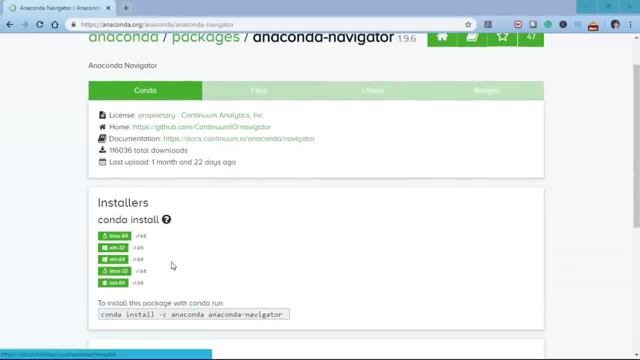 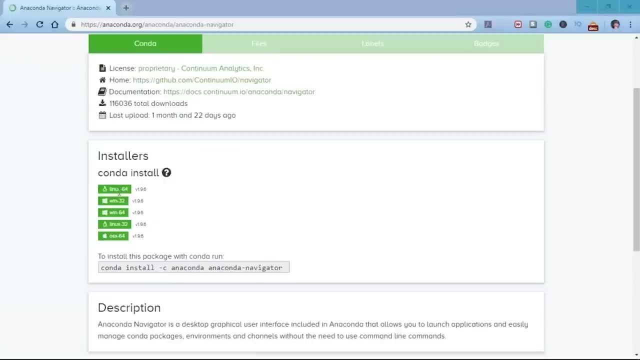 go to anaconda Navigator. So, as you can see, here we have the conda installation code which you're going to use to install it in your particular PC. So either you can use these installers. so once you download the anaconda navigator, it looks something like this: 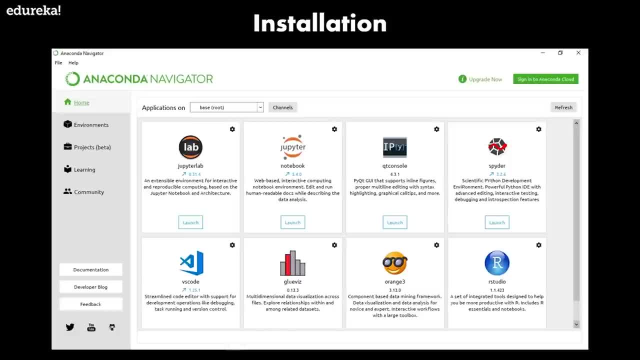 so, as you can see here, we have jupyter lab, jupyter notebook, we have qt console, which is ipython console. we have spider, which is somewhat similar to r studio in terms of python. again, we have r studio also. we have orange 3, we have gluvis and we have vsc code. our focus today would be on 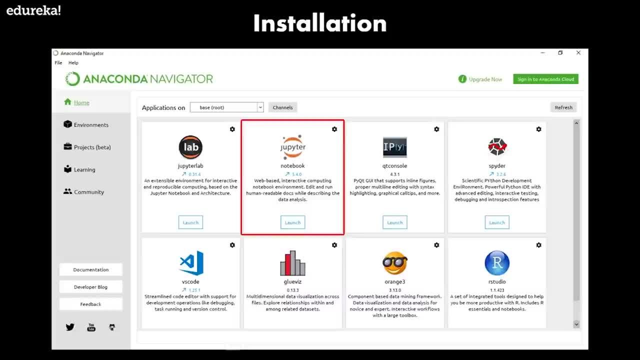 this jupyter notebook itself. now, when you launch the navigator, you can see there are many options available for launching python, as well as our instances now. by definition, a jupyter notebook is fundamentally a json file with a number of annotations. now it has three main parts, which: 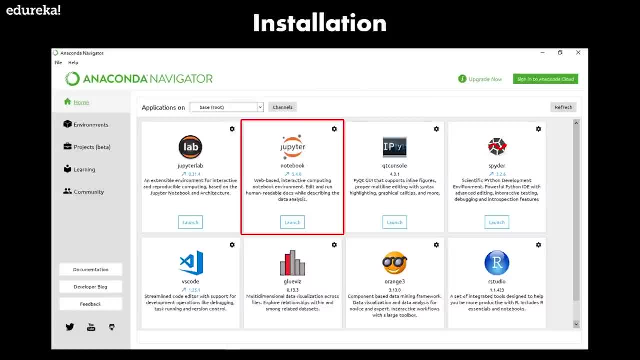 are the metadata, the notebook format and the list of cells. now you should get yourself acquainted with the environment. the jupyter user interface has a number of components, so it's important to know what are components you should be using on a daily basis and you should get acquainted with it. 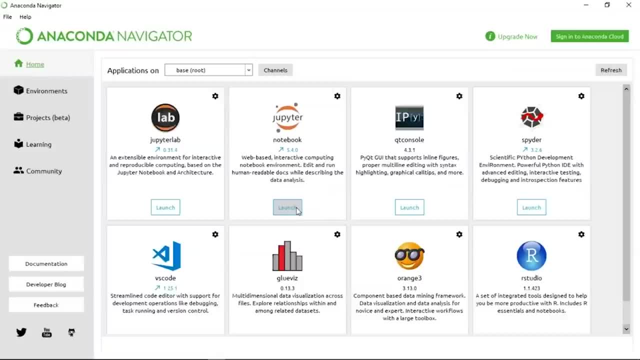 so, as you can see here, our focus today will be on the jupyter notebook. so let me just launch the jupyter notebook now. what it does is creates a online python instance for you to use it over the web. so let it launch now. as you can see, we have jupyter on the top left. 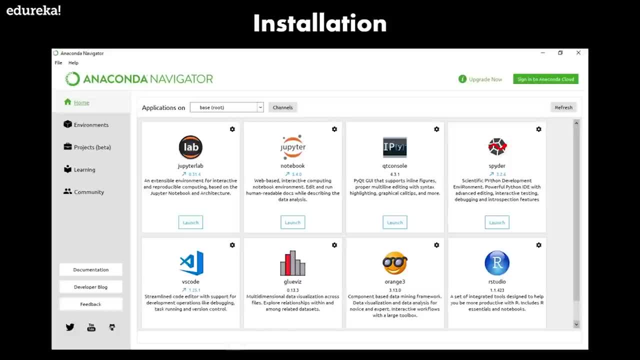 like this. So, as you can see, here we have Jupiter lab, Jupiter notebook, We have cutie console- This is ipython console. We have spider, which is somewhat similar to our studio in terms of python- again, We have our studio. So we have orange three. 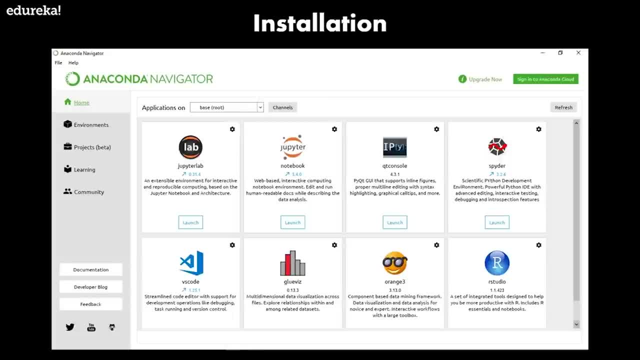 We have glue is and we have VSC code. our focus today would be on this Jupiter notebook itself. Now, when you launch the navigator, you can see there are many options available For launching python, as well as our instances. Now, by definition, a Jupiter notebook is fundamentally adjacent. 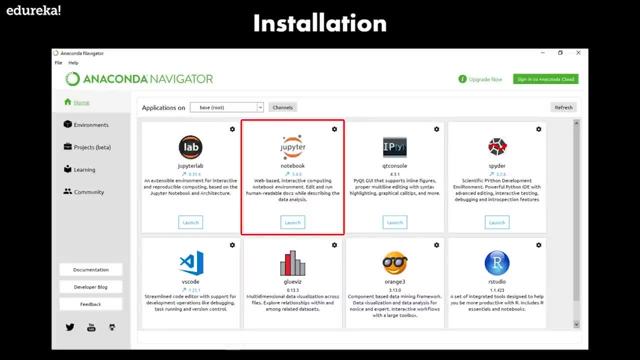 file with a number of annotations. Now it has three main parts, which are the metadata, the notebook format and the list of cells. Now you should get yourself acquainted with the environment. The Jupiter user interface has a number of components, So it's important to know what are components you should be. 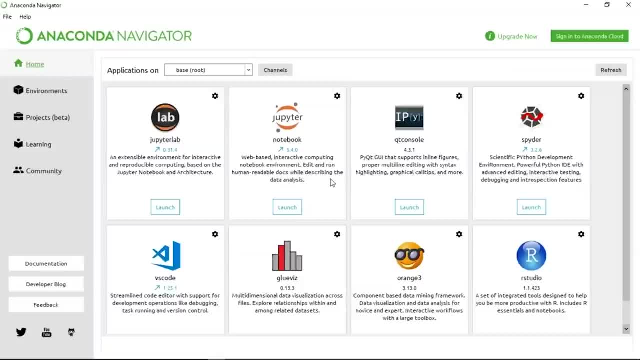 using on a daily basis and you should get acquainted with it. So, as you can see here, our focus today will be on the Jupiter notebook, So let me just launch the trip in a notebook Now. what it does is creates a online python instance for you. 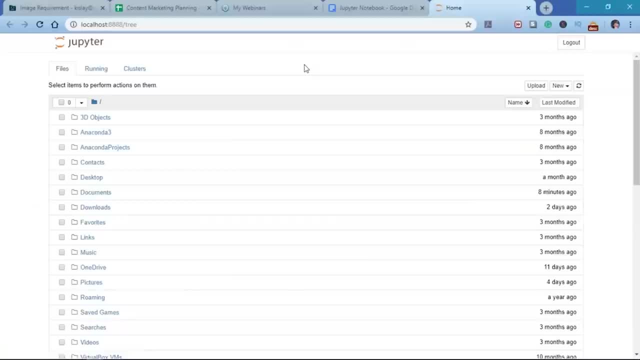 to use it over the web. So let it launch now. As you can see, we have Jupiter on the top left, as expected, and this acts as a button to go to your home page. Whenever you click on this, you get back to your particular. 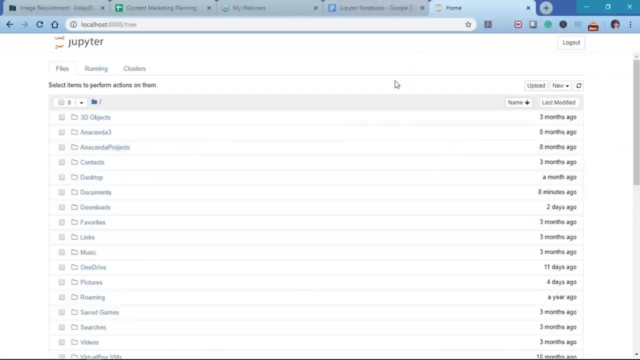 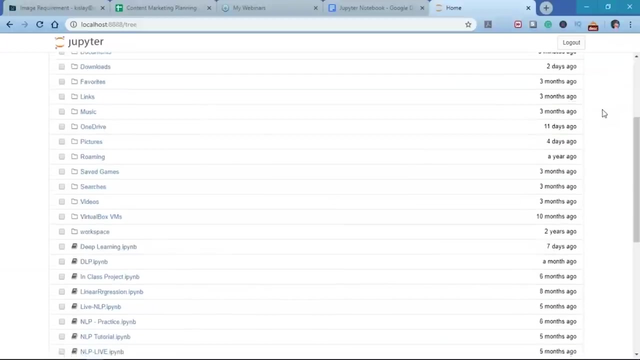 home page. That is the dashboard. Now there are three tabs displayed without the files running and clusters, And what we'll do is we'll understand all of these three and understand what are the importance of these three tabs. or the file tab shows the list of the current files in the directory. 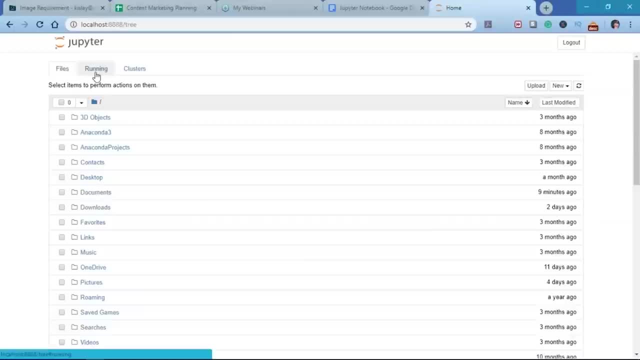 So, as you can see, we have so many files here. Now the running tab presents another screen of the currently running processes and the notebooks. Now the drop-down list for the terminals and notebooks are populated with their running numbers. So, as you can see, inside we do not have any running terminals. 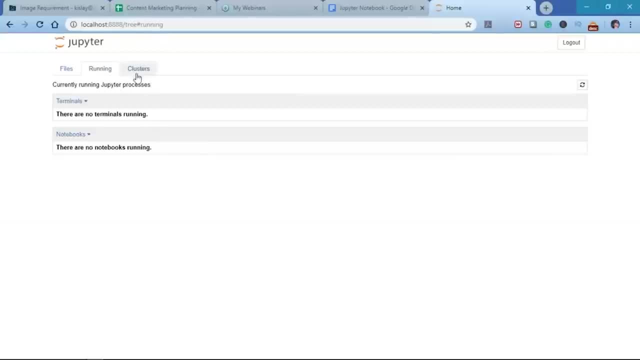 or there are no running notebooks as of now and the cluster tab presents Another screen to display the list of clusters available. in the top right corner of the screen There are three buttons, which are upload, new and the refresh button. Let me go back here. 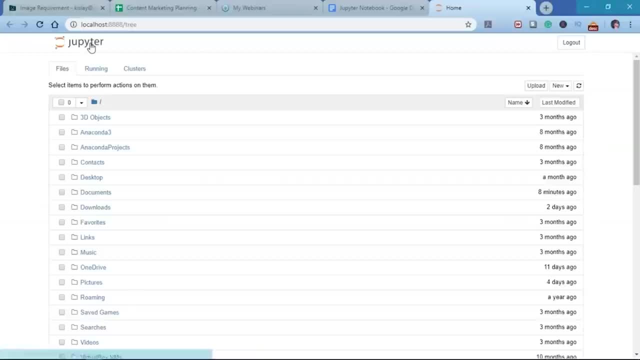 as expected, and this acts as a button to go to your home page. whenever you click on this, you get back to your particular home page. that is the dashboard. now there are three tabs displayed, which are the files, running and clusters, and what we'll do is we'll understand all of these three. 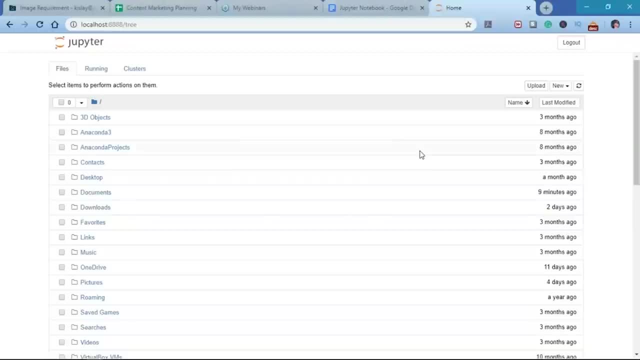 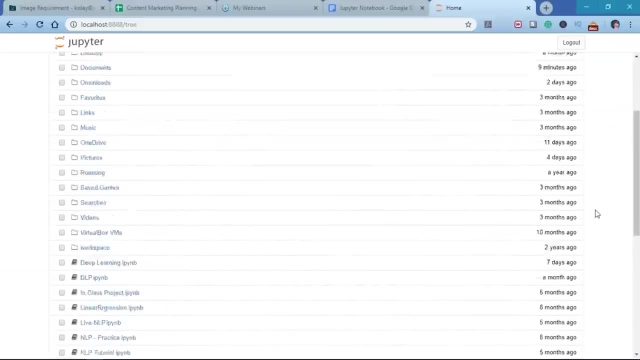 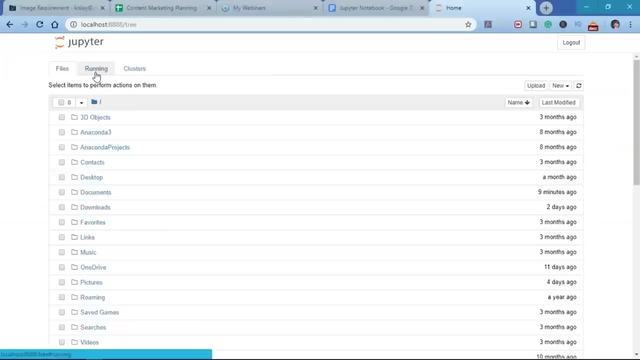 tabs and understand what are the importance of these three tabs. or the file tab shows the list of the current files in the directory. so as you can see, we have so many files here. now. the running tab presents another screen of the currently running processes and the notebooks. now the drop down list. 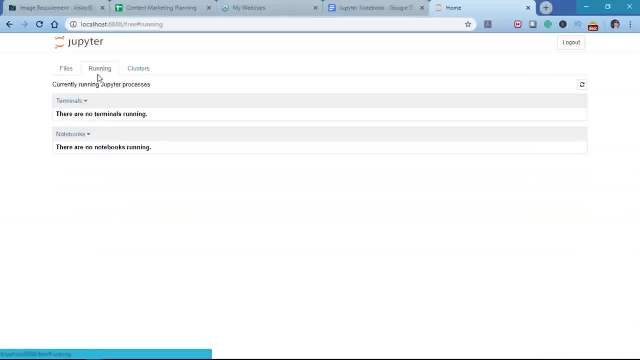 for the terminals and notebooks are populated with their running numbers. so, as you can see inside we do not have any running terminals or there are no running notebooks as of now and the cluster tab presents another screen to display the list of clusters available. so in the top right corner of the screen, 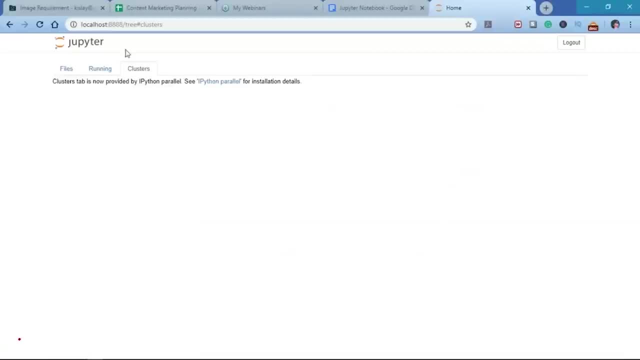 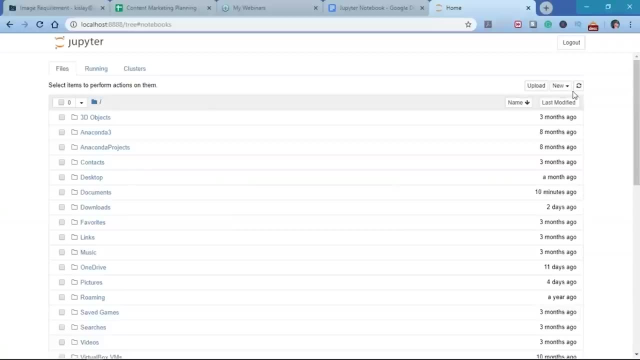 there are three buttons, which are upload, new and the refresh button. let me go back here. so, as you can see, here we have the upload, new and the refresh button. now, the upload button is used to add files to the notebook space, and you may also just drag and drop as you would when handling files. similarly, 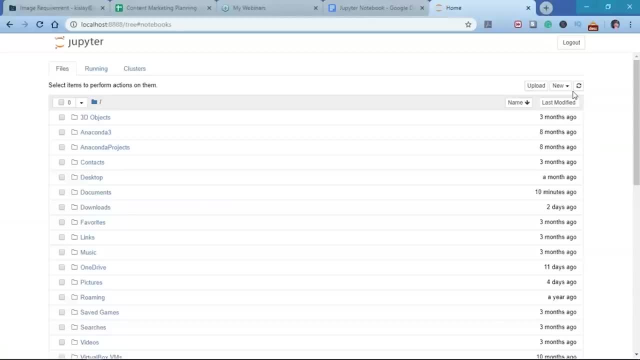 you can drag and drop notebooks into specific folders as well. now the menu with the new in the top presents a further menu of text file folders: terminal and python 3.. now the text file option is used to add a text file to the current directory. now jupyter will open a new browser window for you for the running new text editor. 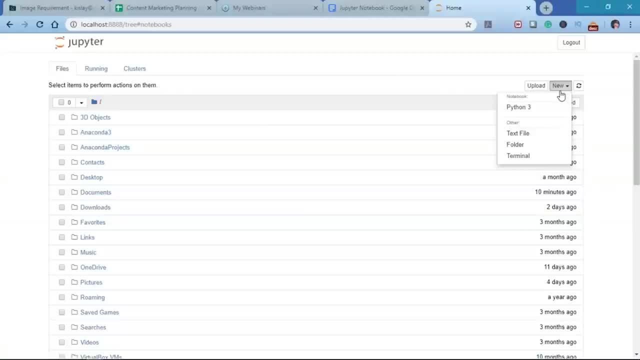 now the text entered is automatically saved and will be displayed in your notebook's files. display now the folder option. what it does is creates a new folder with the name untitled folder. and remember: all the files and folder names are editable. now the terminal option allows you to. 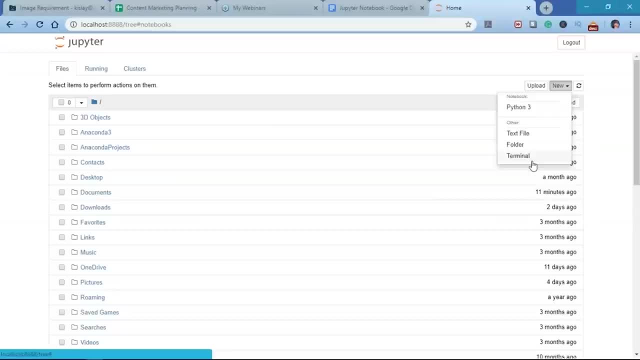 start an ipython session. the notebook options available will be activated when additional notebooks are available in your environment. the python 3 option is used to begin python 3 session interactively in your node. the interface looks like the following screenshot. now what you have is full file editing capabilities. 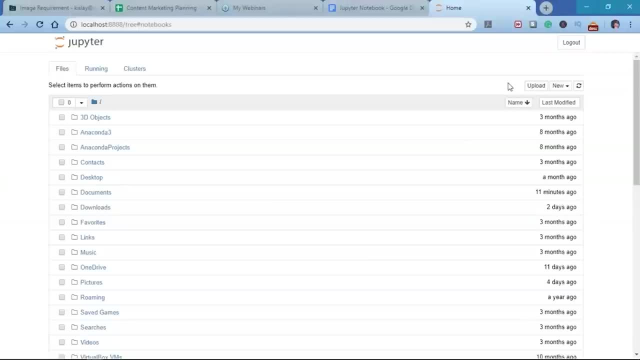 for your script, including saving as new file. you also have a complete working id for your python script now if you come to the refresh button. the refresh button is used to update the display. it's not really necessary, as the display is reactive, to interact with the screen, so you can use it to. 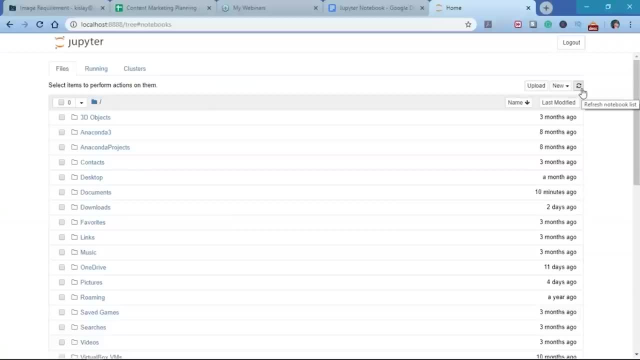 So, as you can see, here we have the upload new and the refresh button. Now the upload button is used to add files to the notebook space and you may also just drag and drop as you would when handling files. Similarly, you can drag and drop notebooks into specific folders. 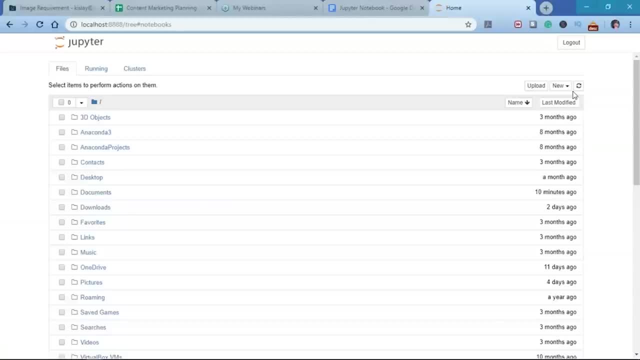 as well. Now the menu with the new in the top presents a further menu of text file Folders: terminal and python 3.. Now the text file option is used to add a text file to the current directory. Now Jupiter will open a new browser window for you for the. 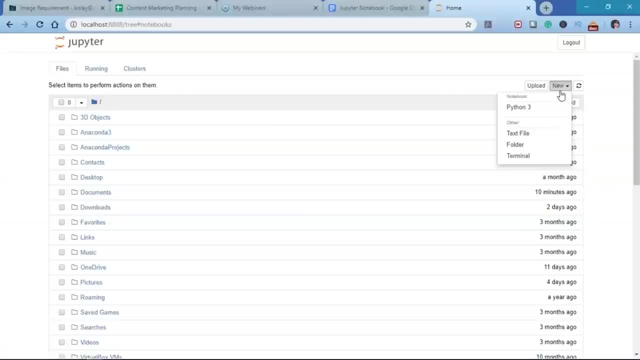 running new text editor. Now the text entered is automatically saved and will be displayed in your notebooks files. display Now the folder option. what it does is creates a new folder with the name untitled folder and remember all the files and folder names are editable. 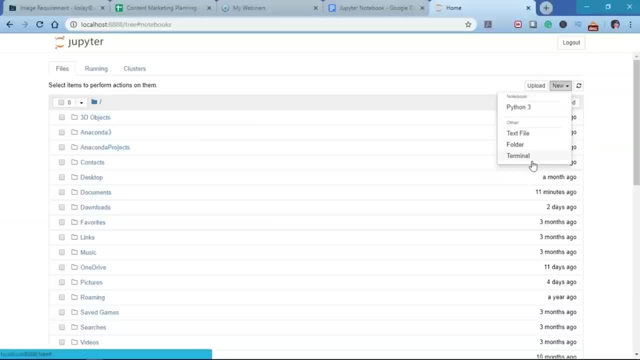 Now the terminal option allows you to start an ipython session. The notebook options available will be activated when additional notebooks are available in your environment. The python 3 option is used to begin python 3 session interactively in your node. The interface looks like the following screenshot. 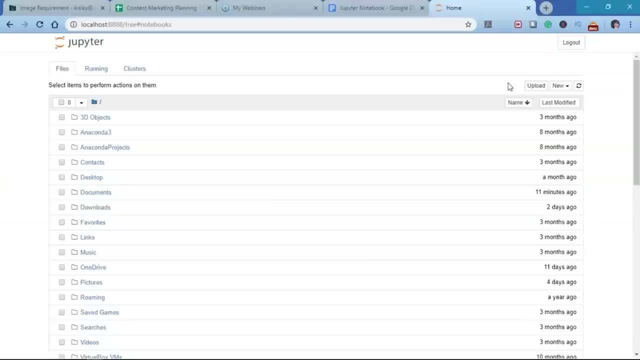 Now what you have is full file editing capabilities for your script, including saving as new file. You also have a complete working ID for your python script. Now if we come to the refresh button. the refresh button is used to update the display. It's not really necessary, as the display is reactivated. 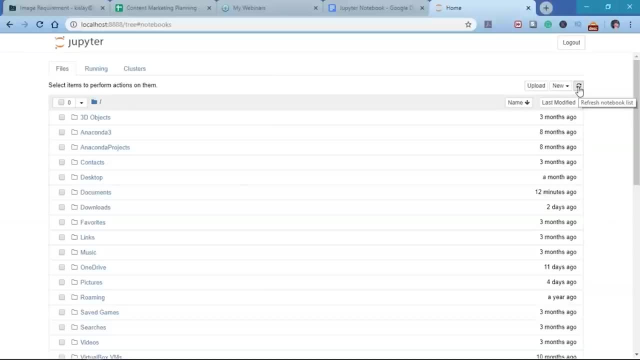 To any changes in the underlying file structure, and at the top of the files tab item There is a checkbox drop down menu and a home button. As you can see, here We have the checkbox, the drop down menu and the home button. Now the checkbox is used to toggle all the checkboxes in the item. 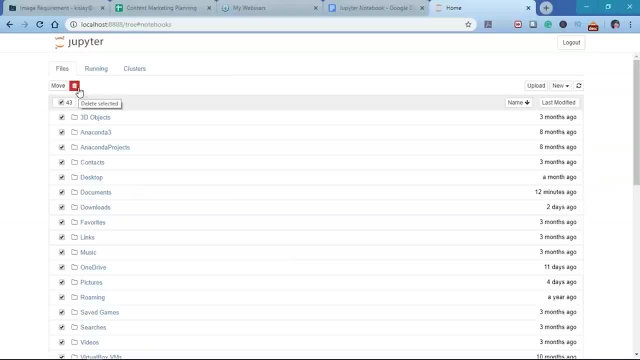 list. So, as you can see, you can select all of these. you can either move or either delete all of the files selected, or what you can do is select all and just select some of the files That's your wish. Now the drop down menu presents a list of choices available, which 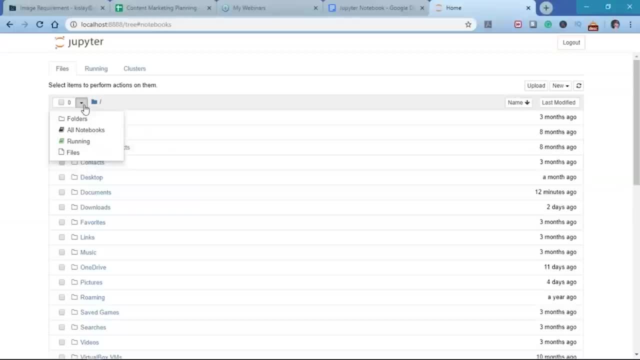 are the folders, All notebooks running and files to the folder section will select all the folders in the display and present a count of the folders in the small box. So as you can see here we have 18 number of folders. Now all the notebook section will change the count of the number. 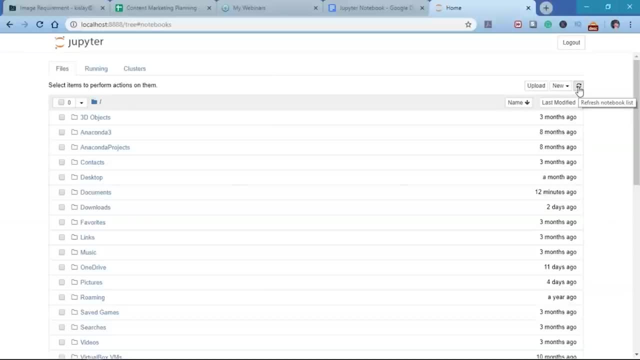 update the screen. so you can use it to update the screen. so you can use it to update the screen. in the underlying file structure and at the top of the files tab item there is a check box, a drop down menu and a home button. as you can see, here we have the check box, the drop down menu and 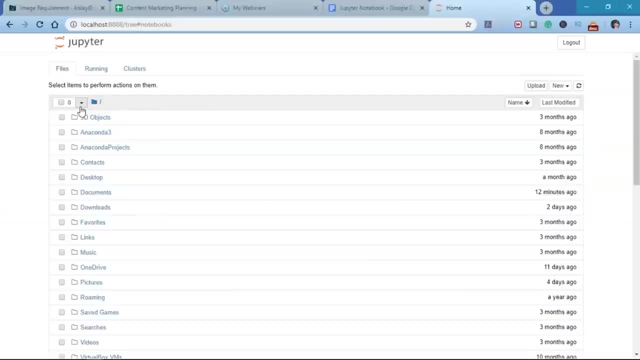 the home button. now the check box is used to toggle all the check boxes in the item list. so, as you can see, you can select all of these. you can either move or either delete all of the files selected, or what you can do is select all and just select some of the files. that's your wish. 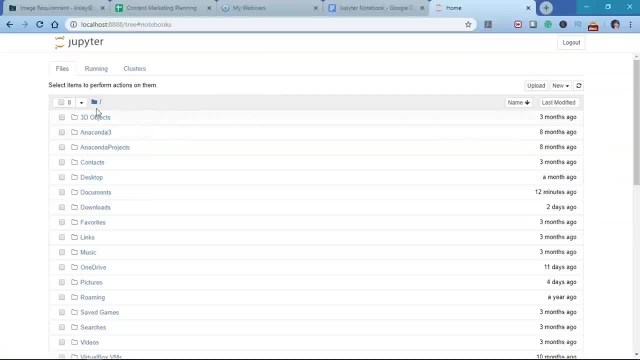 now the drop down menu presents a list of choices available, which are the folders, notebooks, running and files. so the folder section will select all the folders in the display and present a count of the folders in the small box. so as you can see, here we have 18 number of folders. 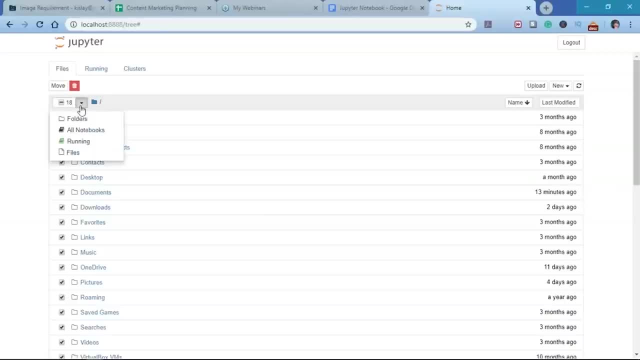 now all the notebook section will change the count of the number of notebooks and provide you with three options. so you can see here it has selected all the given notebooks, which are 18 in number, and you get the option to either duplicate the current notebook- you need to move it. 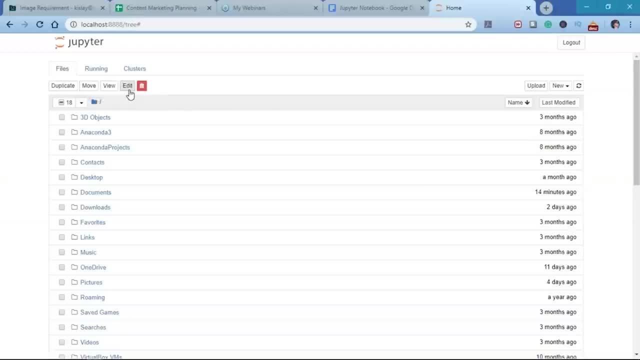 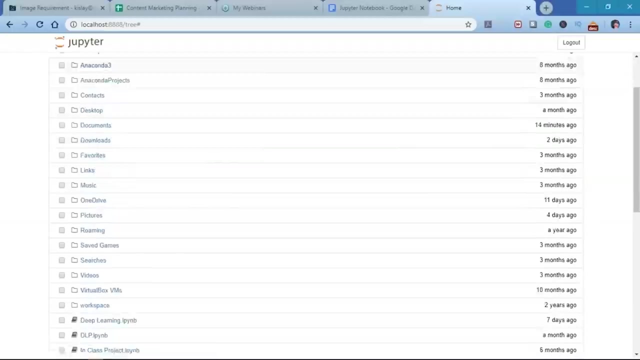 view it, edit it or delete. now the running section will select any running scripts- as you can see, here we have zero running scripts- and update the count to the number selected. now the file section will select all the files in the notebook display and update the accounts accordingly. so if you select the files, here we have seven files, as you can see. 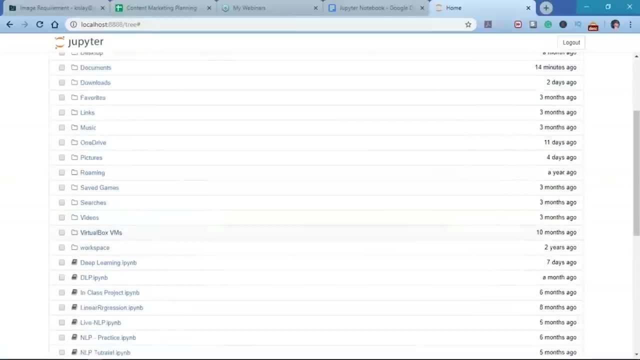 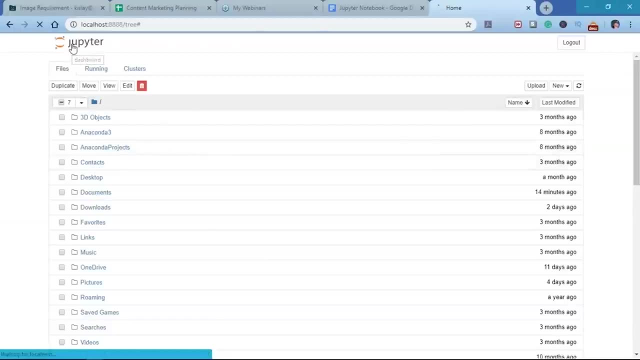 here we have seven files, some data sets, csv files and text files. now the home button brings you back to the home screen of the notebook. so all you need to do is click on the jupyter notebook logo. it will bring you back to the jupyter notebook. 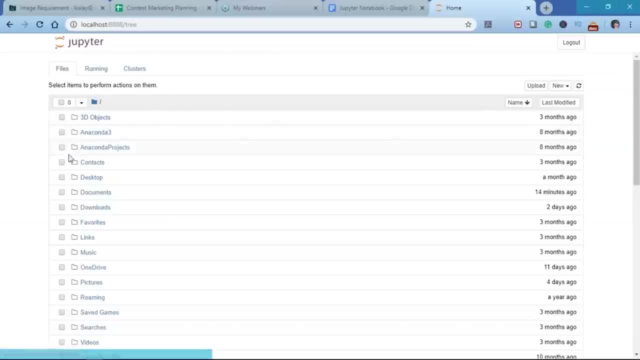 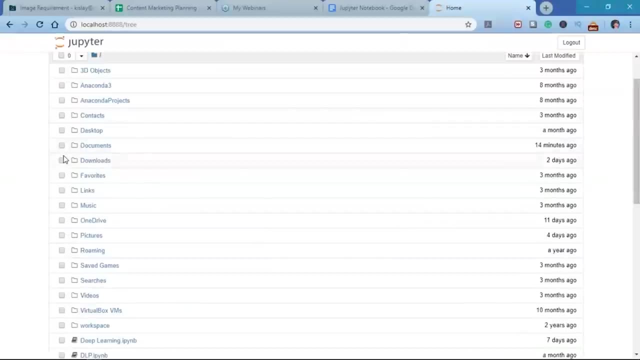 dashboard. now, as you can see, on the left hand side of every item is a checkbox, an icon and the item's name. the checkbox is used to build a set of files to operate upon and the icon is indicative of the type of the item, and in this case, all of the items are folder here. 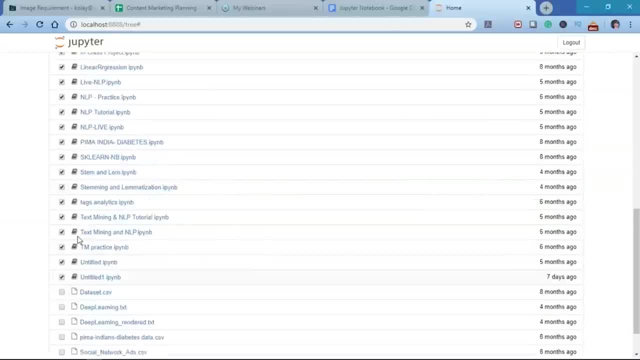 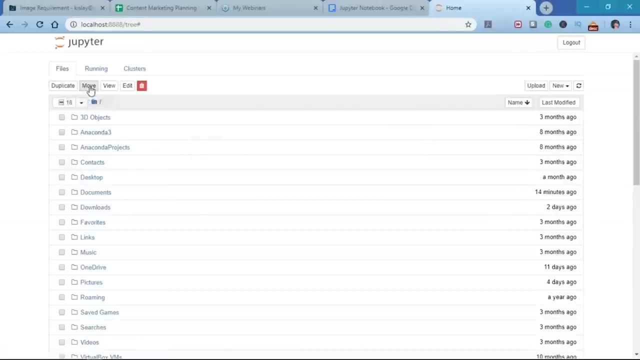 of notebooks and provide you with three option. So you can see here It has selected all the given notebooks, which are 18 a number, and you get the option to either duplicate the current notebook- You need to move it, view it, edit it or delete. 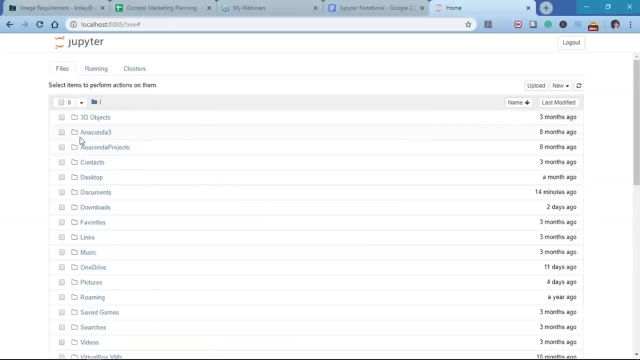 Now The running section will select any running scripts- as you can see, here We have zero running scripts- and update the count to the number selected. Now the file section will select all the files in the notebook display and update the counts accordingly. So if you select the files, here we have seven files as you can. 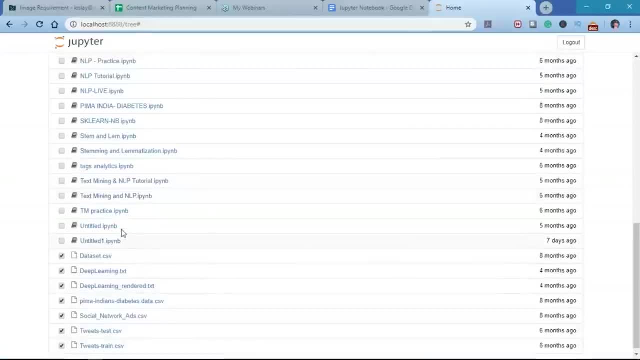 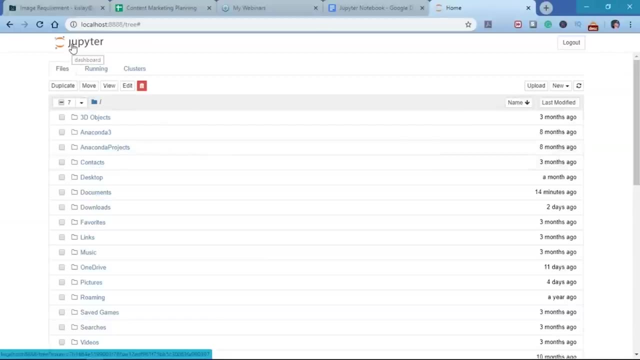 see here We have seven files, some data sets, CSE files and text files. Now the home button brings you back to the home screen of the notebook, So all you need to do is click on the Jupiter notebook logo. It will bring you back to the 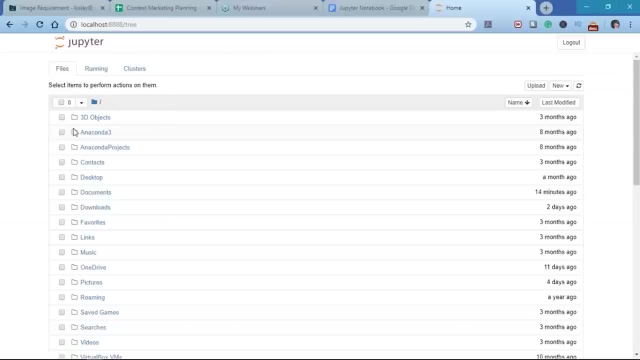 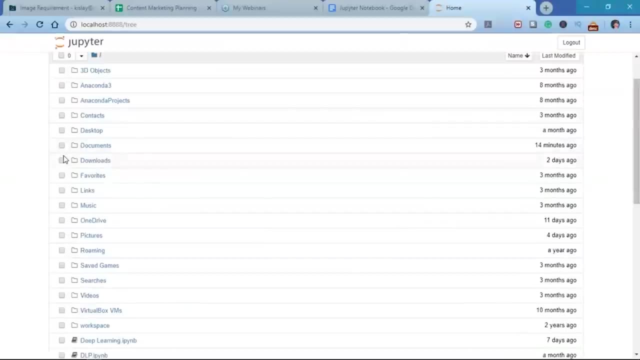 Jupiter notebook dashboard. Now, as you can see, on the left hand side of every item is a checkbox and I can and the items name. the checkbox is used to build a set of files to operate upon and the icon is indicative of the type of the item and in this case, all of the items are folder here. 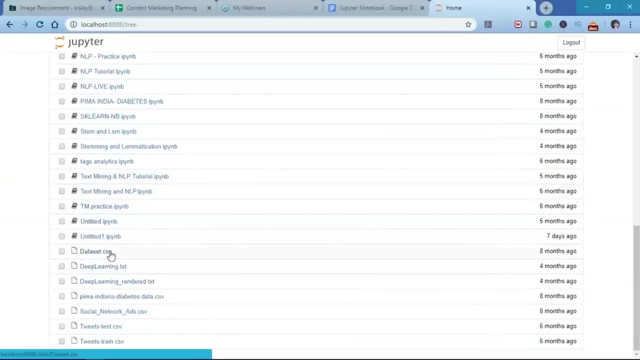 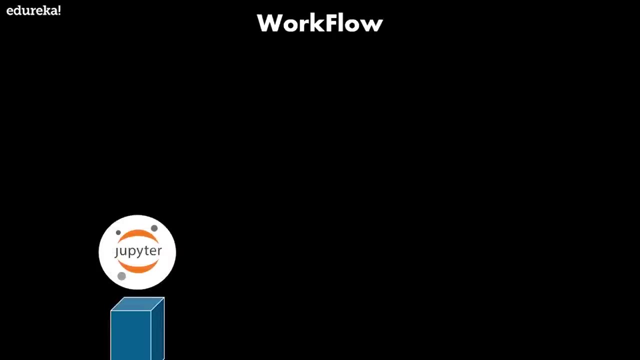 coming down. We have the rain notebooks and finally, we have certain files, which are the text files and the CSV files. Now, a typical workflow of any Jupiter notebook is to first of all, create a notebook for the project or your data analysis, Add your analysis, step coding and output and surround your 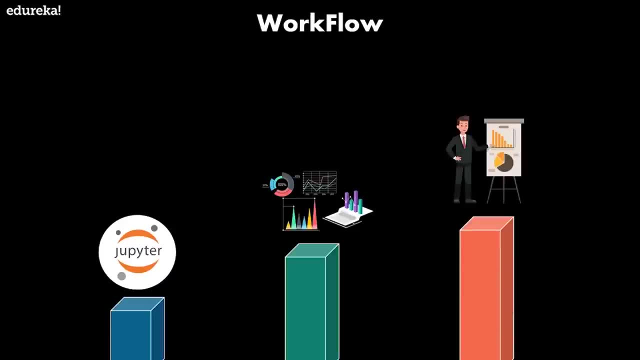 analysis, with organization and presentation Markdown to communicate an entire story. Now, interactive notebooks that include widgets and display modules would then be used by others, by modifying parameters and the data, to note the effects of the changes. Now, if we talk about security, Jupiter notebooks are created in. 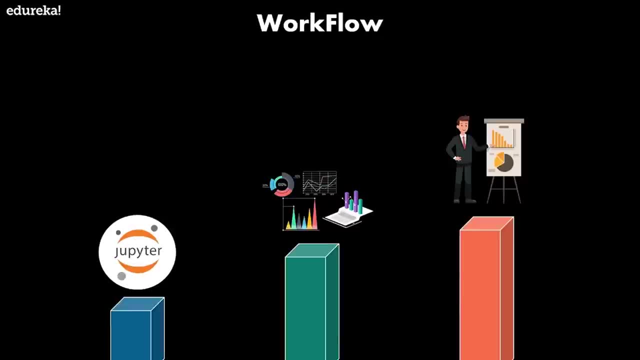 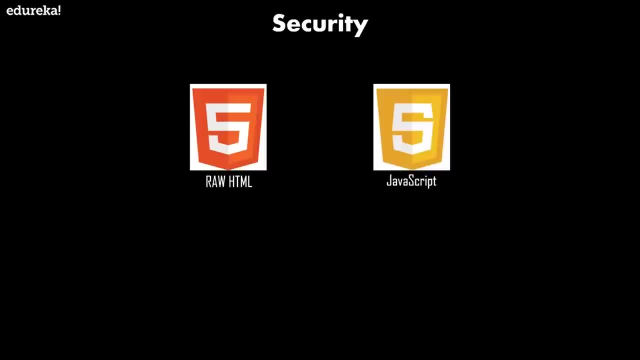 order to be shared with other users, in many cases, over the internet. However, Jupiter notebook can execute arbitrary code and generate arbitrary code. This can be a problem If malicious aspects have been placed in the note. now, the default security mechanism for Jupiter notebooks include raw HTML, which. 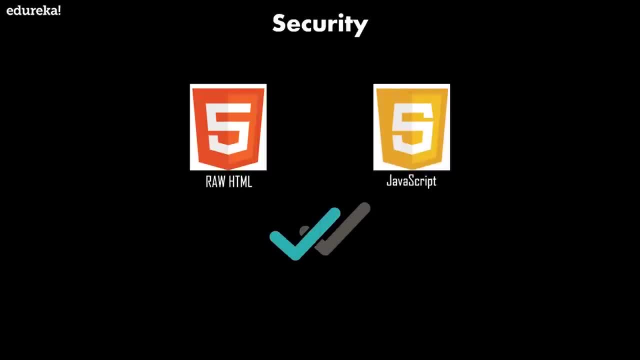 is always sanitized and checked for malicious coding. Another aspect is you cannot run external JavaScript's. another cell contents, especially the HTML and the JavaScript's, are not trusted. It requires user validation to continue and the output from any cell is not trusted. all of the HTML or JavaScript is never trusted and 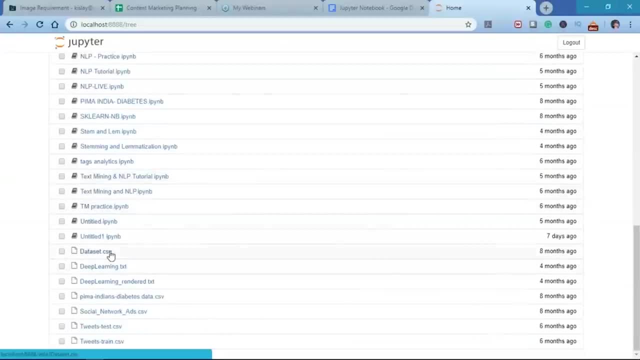 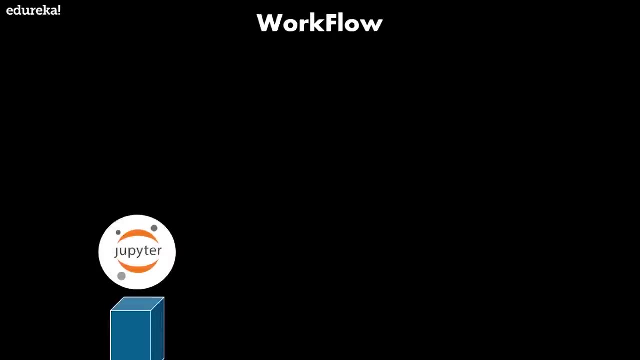 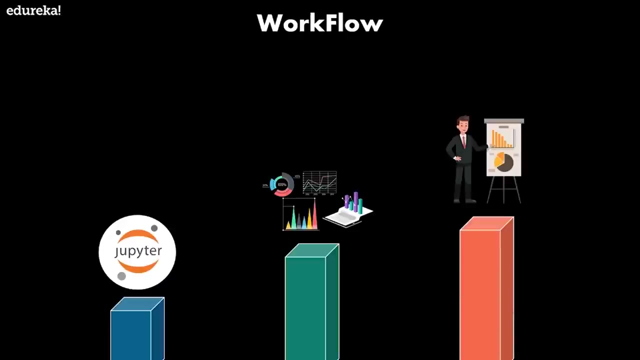 coming down, we have the running notebooks and finally we have certain files, which are the text files and the csv files. now a typical workflow of any jupyter notebook is to first of all create a notebook for the project or your data analysis, step coding and output and surround your analysis with organization and presentation markdown. 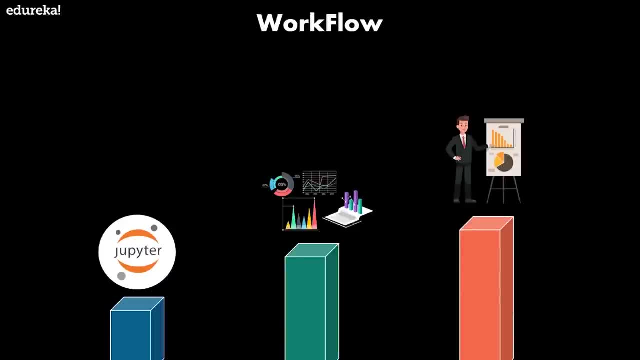 to communicate an entire story now. interactive notebooks that include widgets and display modules would then be used by others, by modifying parameters and the data, to note the effects of their changes. now, if we talk about security, jupyter notebooks are created in order to be shared with other users, in many cases, over the internet. however, jupyter notebook 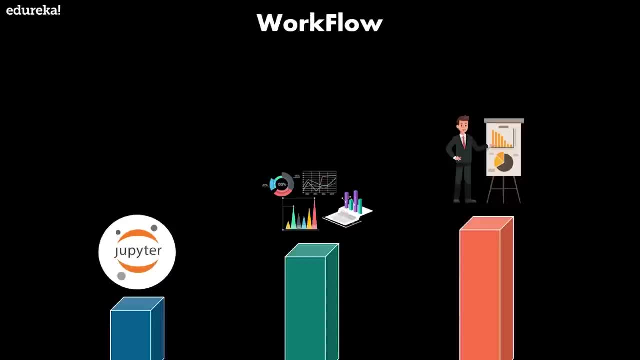 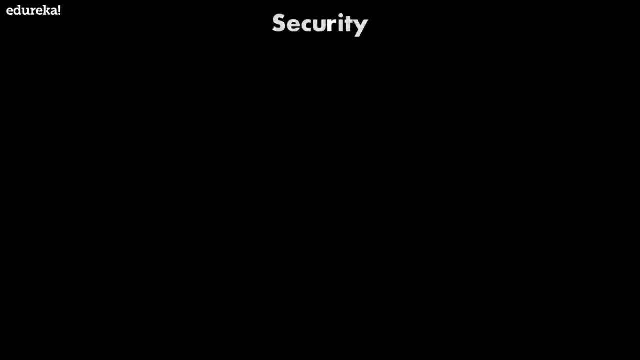 can execute arbitrary code and generate arbitrary code. this can be a problem if malicious aspects have been placed in the notebook. now the default security mechanism for jupyter notebooks include raw html, which is always sanitized and checked for malicious coding. another aspect is you cannot run external javascripts now the cell contents especially. 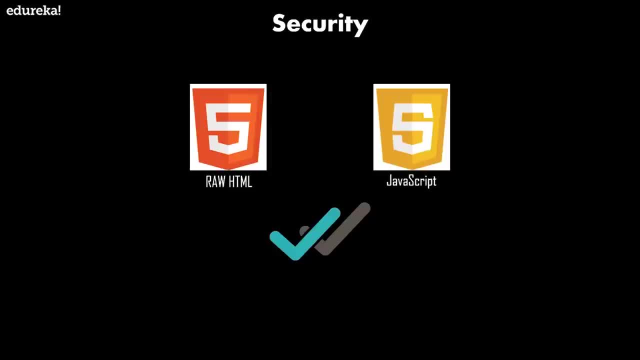 the html and the javascripts are not trusted. it requires user validation to continue and the output from any cell is not trusted. all other html or javascript is never trusted and clearing the output will cause the notebook to break. become trusted when saved. now notebooks can also use a security digest to ensure the correct user. 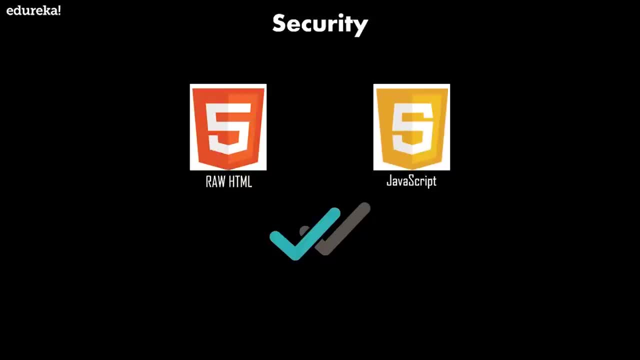 is modifying the contents, so for that, what you need to do is a digest. what it does is takes into the account the entire contents of the notebook and a secret which is only known by the notebook creator. now, this combination ensures that malicious coding is not going to be added to the notebook. 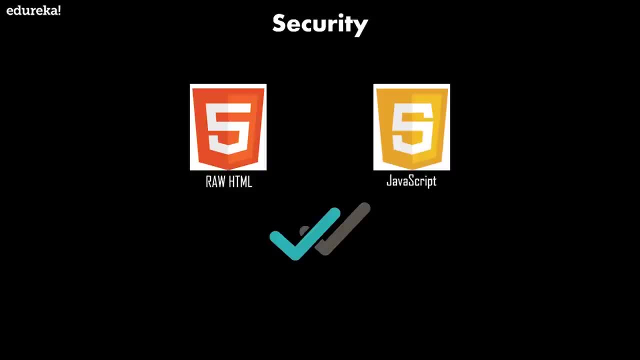 so you can add security digest to notebook using the following command, which i have given here. so it's jupyter, the profile, what you have selected, and inside what you need to do is security and notebook secret. so what you can do is replace the notebook secret with your part of secret and that will act as a key for the 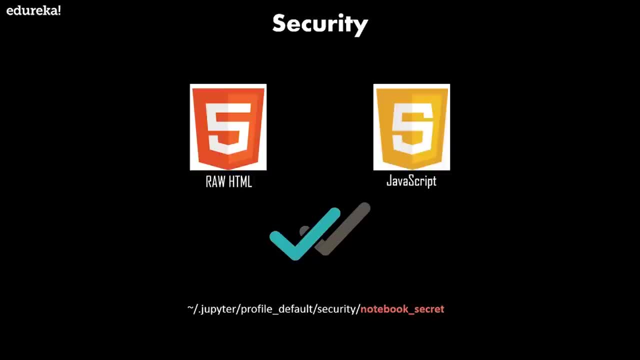 particular notebook. so what you need to do is share that particular key with all your colleagues or whoever you want to share that particular notebook with, and in that case it keeps the notebook secured and away from other malicious coders and all. another aspect of jupyter is: 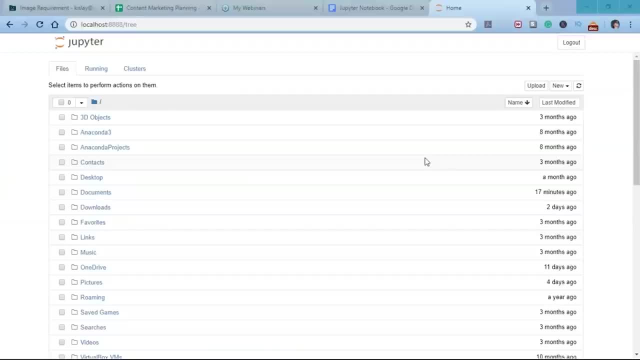 configuration so you can configure some of the display parameters used when presenting notebooks. now, these are configurable due to the use of product known as code mirror to present and modify the notebook. so code mirror, what it basically is, it is a javascript based editor for the use within the web pages and notebooks. so what you do is what you do: code mirror. 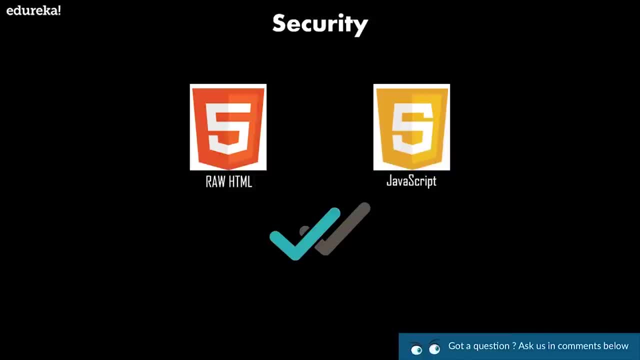 clearing the output Cause the notebook to become trusted when safe. now notebooks can also use a security digest to ensure the correct user is modifying the contents. So for that, what you need to do is a digest. what it does is takes into the account the entire contents of the notebook and a secret. 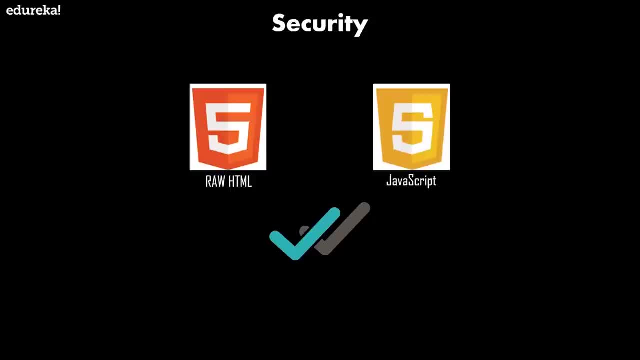 which is only known by the notebook creator, and this combination ensures that malicious coding is not going to be added to the notebook. So you can add security digest to notebook using the following command, which I have given here. So it's Jupiter, The profile, what you have selected, and inside what you need to do is 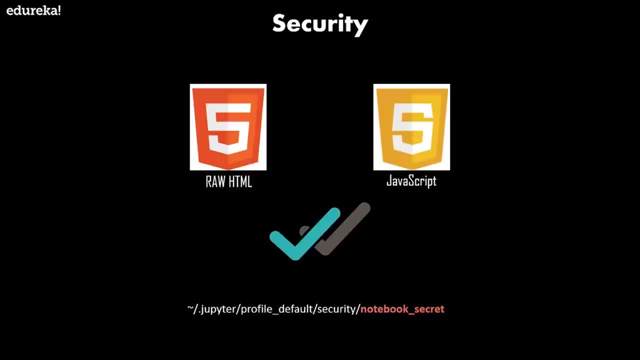 security and notebook secret. So what you can do is replace the notebook secret with your part of secret and that will act as a key for the particular notebook. So what you need to do is share that particular key with all your colleagues or whoever you want to share that particular notebook with. 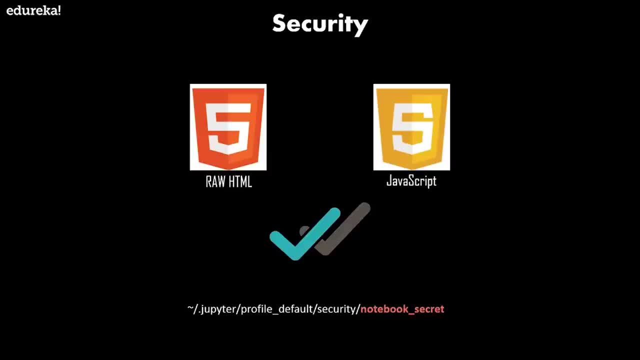 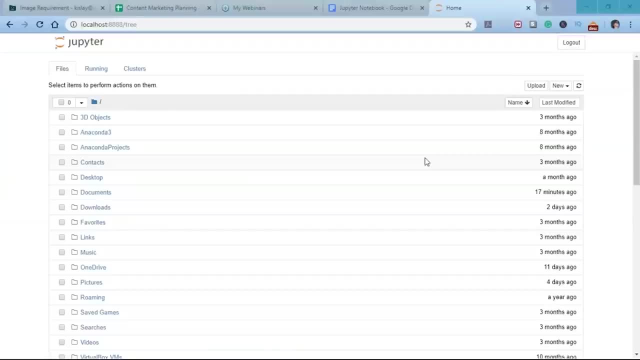 and, in that case, keeps the notebook secured and away from other malicious coders and all other aspect of Jupiter is configuration, so you can configure some of the display Parameters used and presenting notebooks. Now these are configurable due to the use of product known as code. 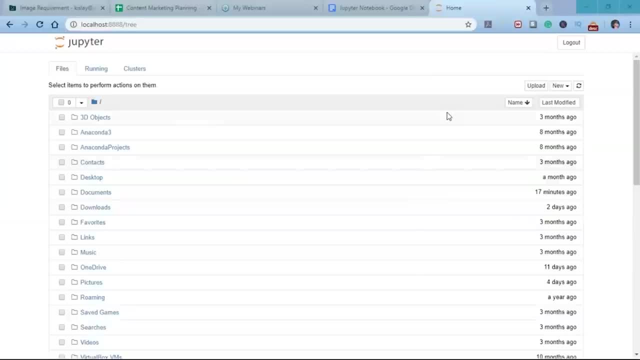 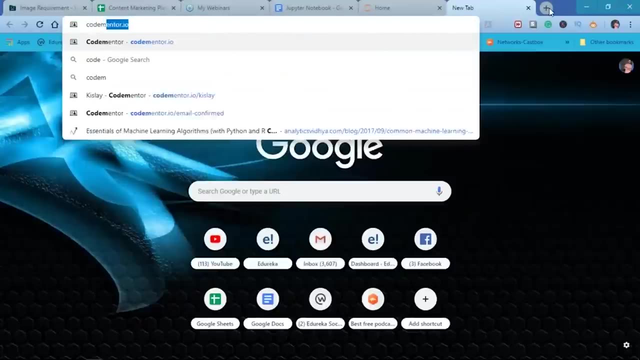 mirror to present and modify the notebook. So code mirror what it basically is, It is a JavaScript based editor for the use within the web pages and notebook. So what you do is what you do: code mirror. So, as you can see here, code mirror is a versatile text editor implemented. 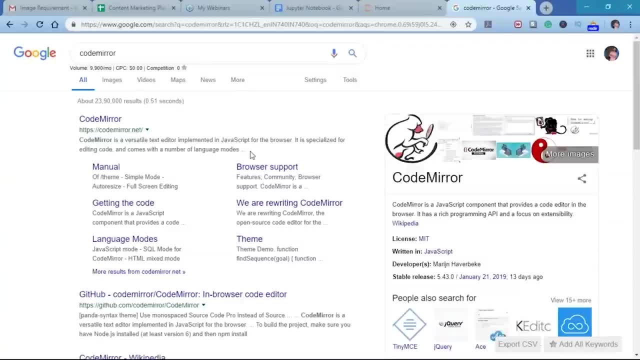 in JavaScript for the browser. So what it does is allow you to configure the options for Jupiter. So now let's execute Some python code and understand the notebook in a better way. Jupiter does not interact with the scripts as much as it executes your. 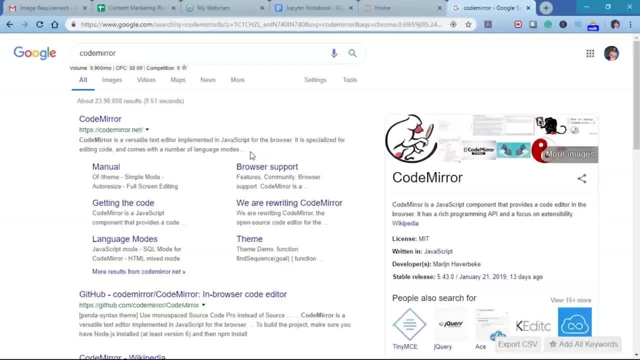 script and records the result. So I think this is how Jupiter notebooks have been extended to other languages besides python, as it just takes a script, runs it against a particular language engine and across the output from the engine, all the while not really knowing what kind of a script is being executed. 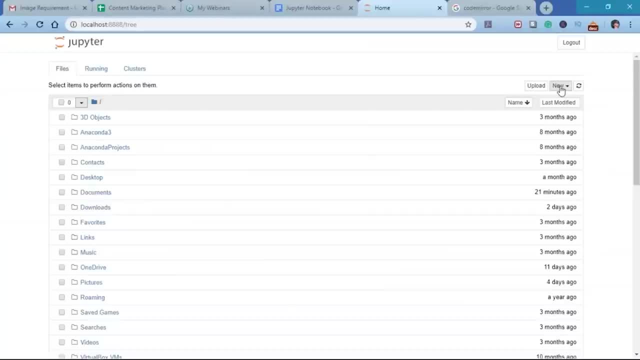 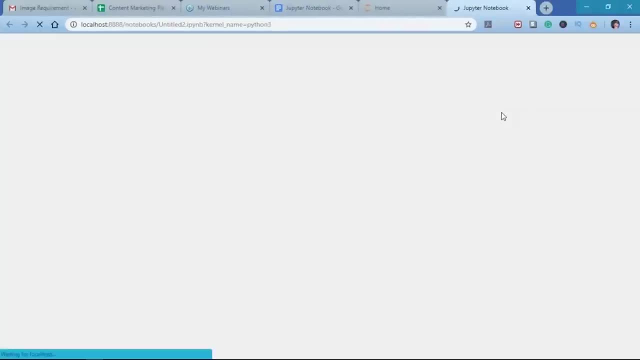 Now the new window shows an empty cell for you to enter the python Code. know what you need to do is, under new, you select the python 3 and what it will do is open a new notebook. Now this notebook is untitled, So let's give the new work area a name: python code. 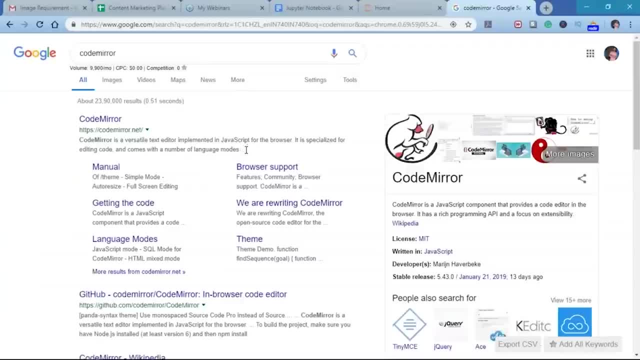 so, as you can see here, code mirror is a versatile text editor implemented in javascript for the browser, so what it does is allow you to configure the options for jupyter. so now let's execute some code and understand the notebook in a better way. jupyter does not interact with your scripts, as 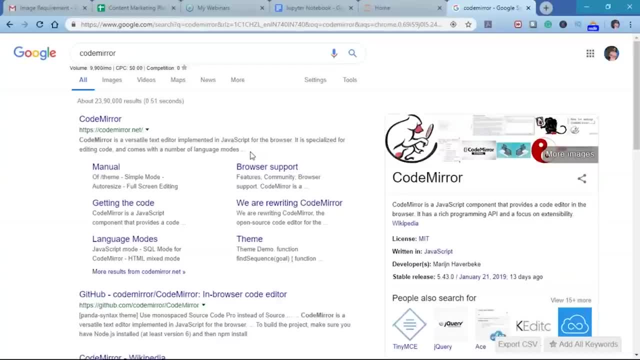 much, as it executes your script and records the result. so i think this is how jupyter notebooks have been extended to other languages besides python, as it just takes a script, runs it against a particular language engine and across the output from the engine, all the while not really knowing. 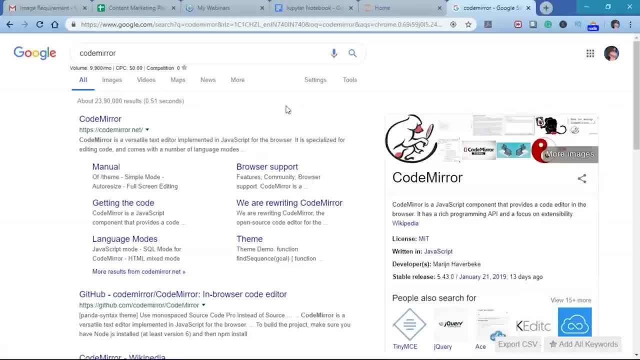 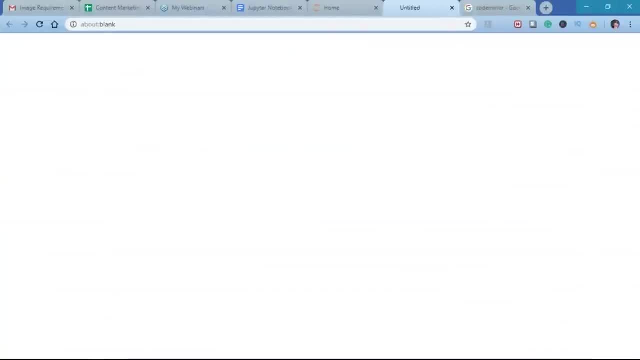 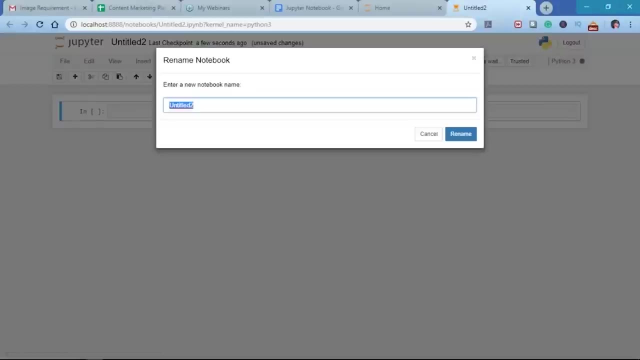 what kind of a script is being executed now? the new window shows an empty cell for you to enter the python code. now what you need to do is, under new, you select the python 3 and what it will do is open a new notebook. now this notebook is untitled, so let's give the new work area a name: python code. so 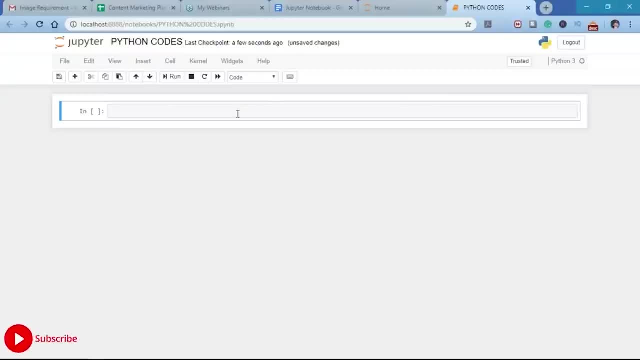 so, as you can see, we have renamed this particular cell. now auto save option should be on the next to the title. as you can see, last checkpoint a few days ago- unsaved changes. the auto save option is always on. what we do is with an accurate name we can find the selection. 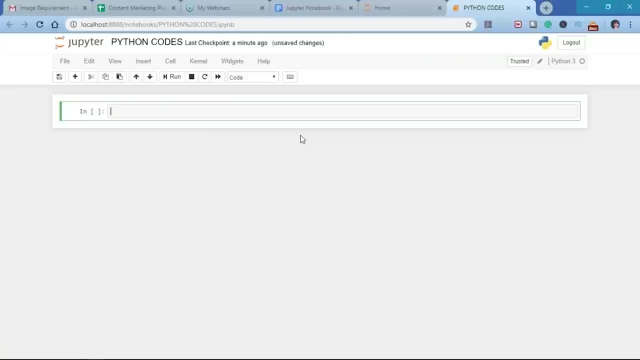 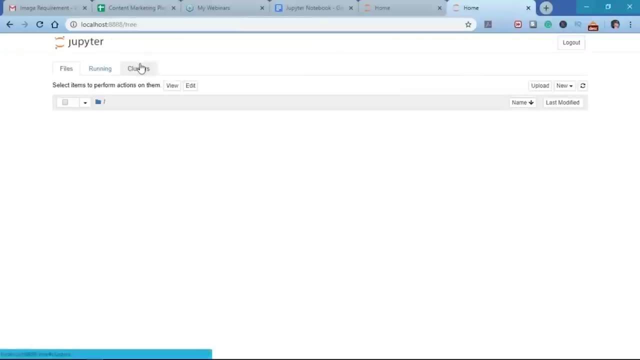 and this particular notebook very easily from the notebook home page. so if you select your browser's home tab and refresh, you will find this new window name displayed here again. so if you just go to the notebook home and, as you can see, i mentioned it, python codes, and under running also, you have the 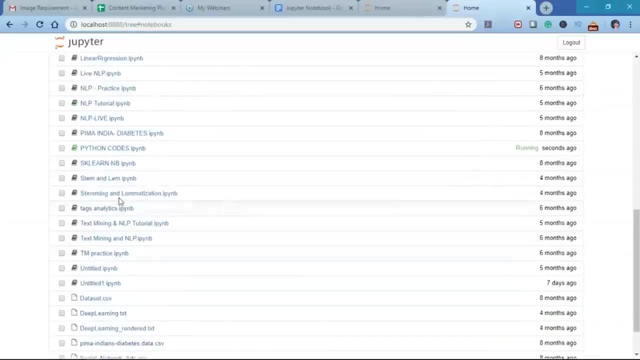 python codes here. so let's get back to the particular page or the notebook. one thing to note here: that it has, and there's an item icon versus a folder icon, the automatically assigned to the directory, and the directory is the ipy and b the ipython node. and since the item is in a browser, 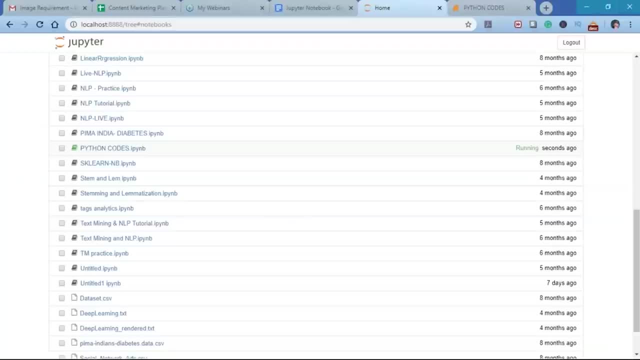 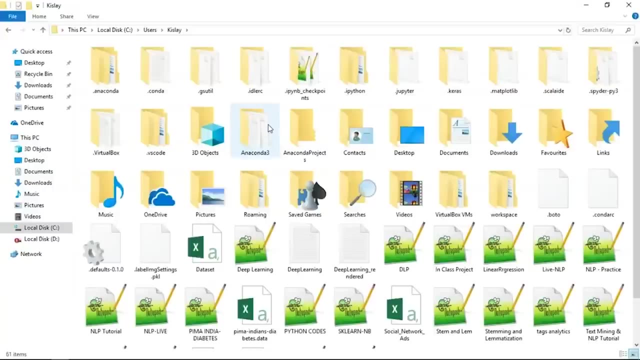 in a jupyter environment. it is marked as running and there is a file by that name in your directory as well. so if you go to your directory, let me go and check it so as you can see, if you go into the users here you can see we have the interest projects, the python codes, so you can see we. 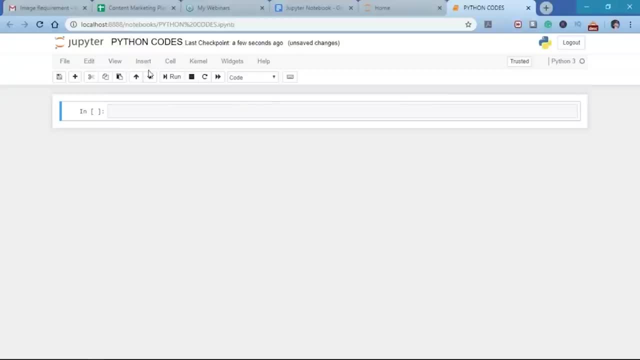 So so, as you can see, we have renamed this particular cell. now, auto save option should be on the next to the title. as you can see, last checkpoint a few days ago: unsaved changes. The auto save option is always on. what we do is with an accurate name. we 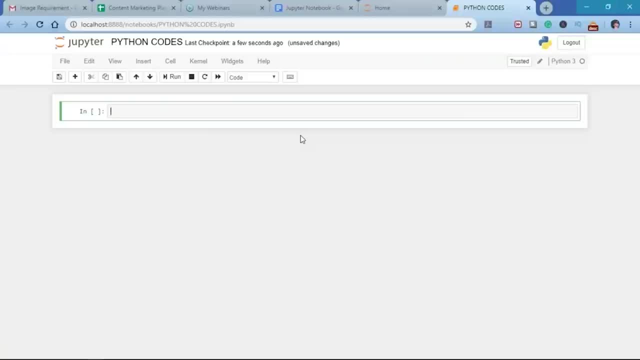 can find the selection and this particular notebook very easily from the notebook home page. So if you select your browser's home tab and refresh, you will find this new window name displayed here again. So if you just go to the notebook home and as you can see, I mentioned it. 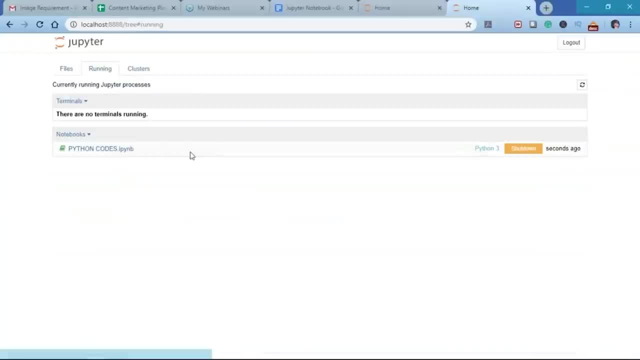 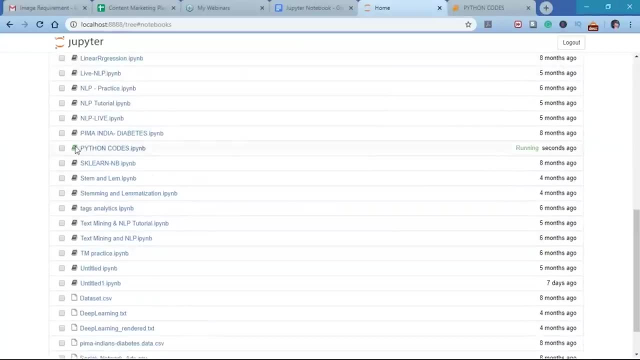 python codes and under running also, you have the python codes here. So let's get back to the particular page or the notebook. one thing to note here: that it has and doesn't item icon versus a folder I can Automatically assigned extension, as you can see here is ipy and be the 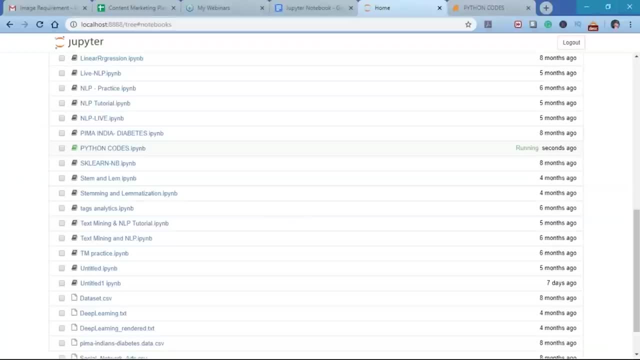 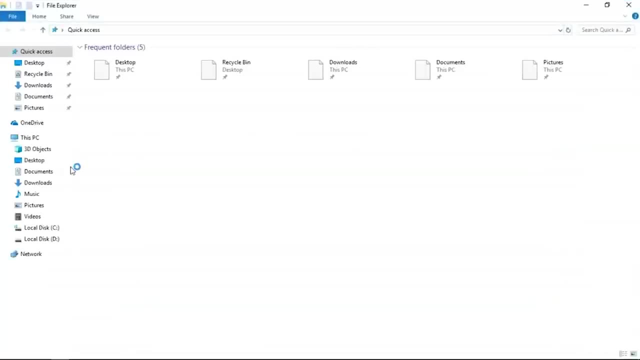 ipython note and says: the item is in a browser in a Jupiter environment. It is marked as running and there is a file by that name in your directory as well. So if you go to your directory, let me go and check it So as you can see, if you go into the users here you can see we have the. 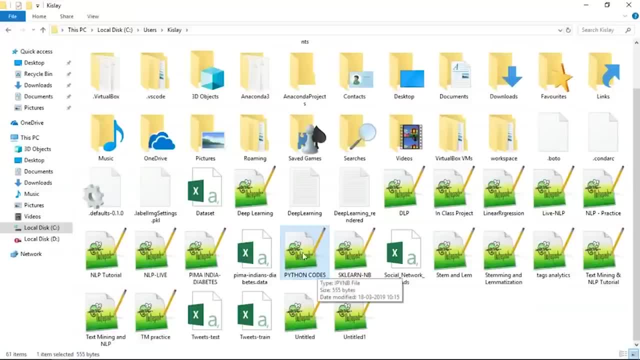 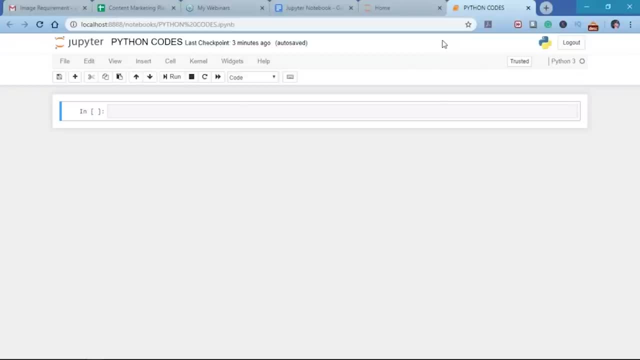 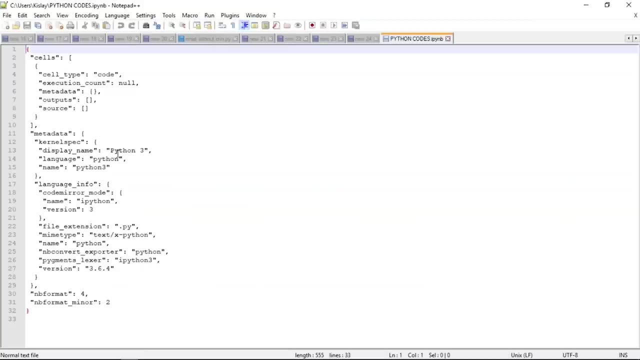 interest projects, the python codes that you see. we automatically have that particular ipython notebook created in our working environment and the local folder space also. So if you open the ipynb file in the text editor you will see basic context of a Jupiter code. as you can see, if I'm opening it, the cells are empty. 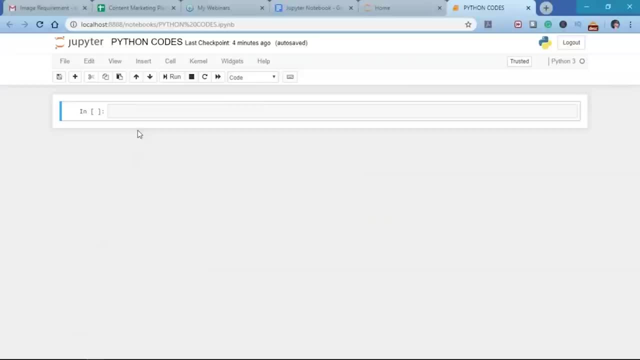 nothing is there, So let's type in some code here. So, for example, I'm going to put in name equals edureka. next, What I'm going to do is provide subscribers that equals 700k And to run this particular cell. 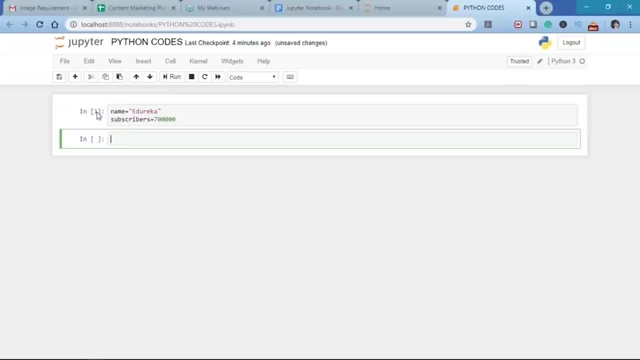 What you need to do is click on the run icon. as you can see here We have one, So this is the first cell to be executed. in the second cell We enter python code that references the variables from the first cell. So, as you can see, here we have friend name. has string subscribers. 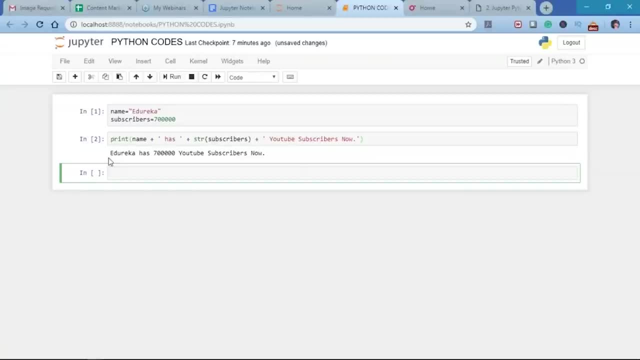 So let me just run this particular so, as you can see here, note that we have an output here that edureka has 700k YouTube subscriber now, so it's more than 700k. now to know more About Jupiter and other Technologies, What you can do is subscribe to our channel and get updates on the latest. 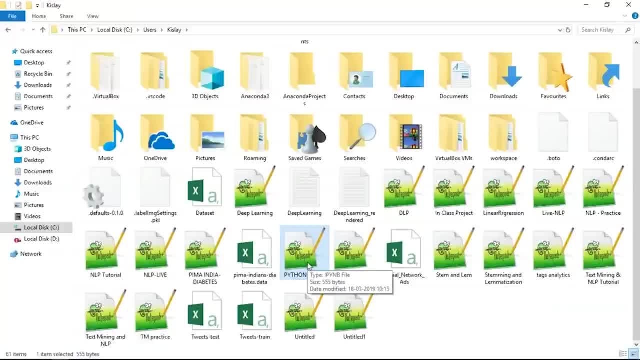 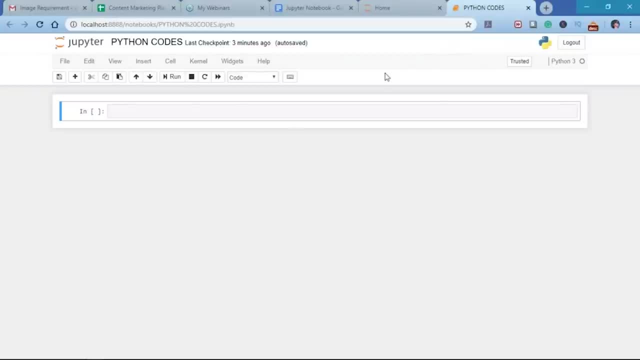 automatically have that particular ipython notebook created in our working environment and the local disk space also. so if you open the ipython code you can see that it's running the ipy and b file. in the text editor you will see basic context of a jupyter code, as you can see. 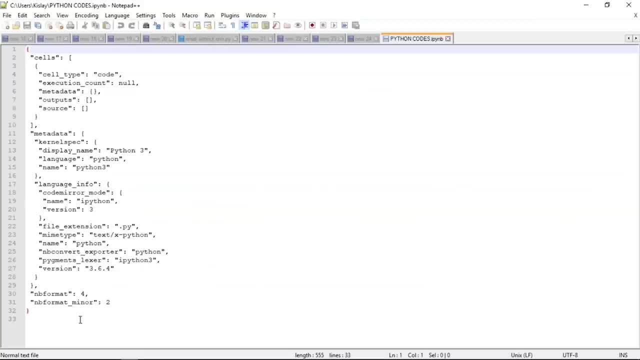 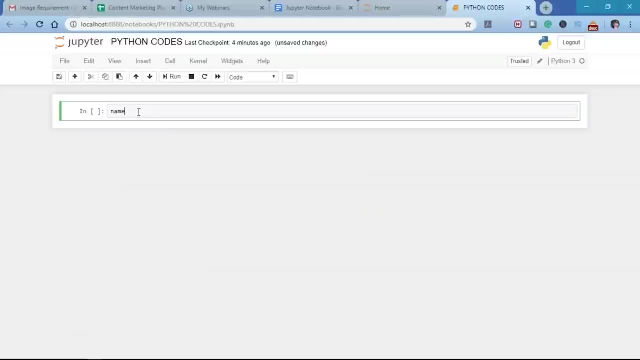 if i'm opening it, the cells are empty. nothing is there. so let's type in some code here. so, for example, i'm going to put in name equals edureka. next, what i'm going to do is provide subscribers. that equals 700k and to run this particular cell. what you need to do is 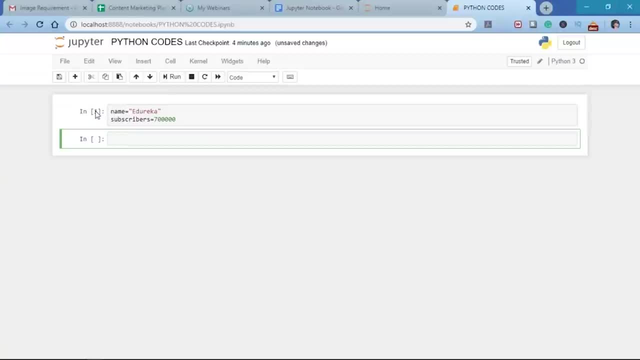 click on the run icon. as you can see, here we have one, so this is the first cell to be executed. in the second cell we enter python code that references the variables from the first cell. so, as you can see, here we have print name, has string subscribers, so let me just run this. 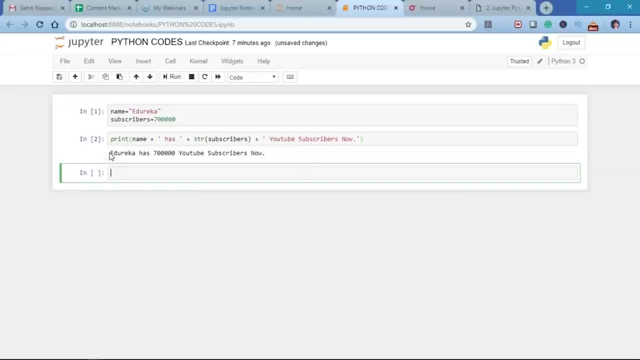 particular. so, as you can see here, note that we have an output here that edureka has 700k youtube subscriber now, so it's more than 700k. now to know more about jupyter and other technologies, what you do is subscribe to our channel and get updates on the latest trending technologies. so note that. 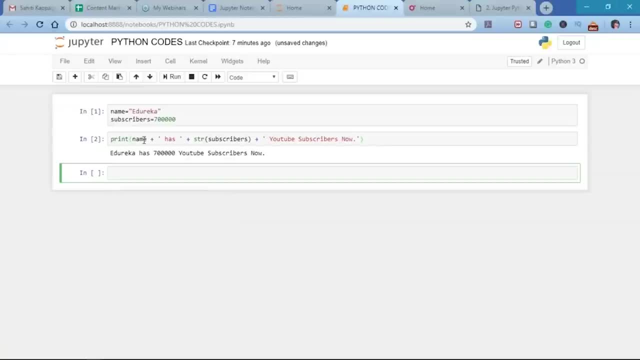 jupyter color codes your python, just as a decent editor would, and we have empty braces to the left of each code block. so, as you can see here, if we execute the cell, the results are displayed in line. now it's interesting that jupyter keeps track of the output last generated in the saved version of. 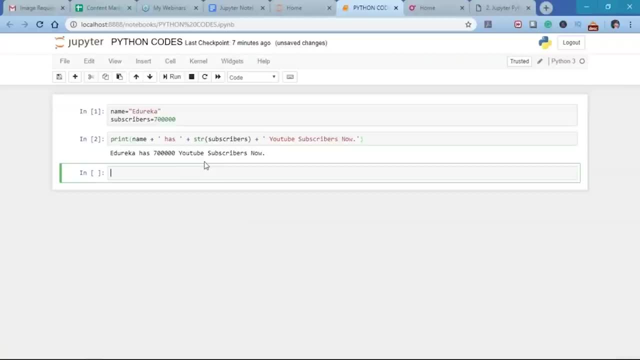 the file and is a safe checkpoints. now, if you were to rerun your cells using the rerun or the run, all the output would be generated and saved by autosave. now the cell number is incremented and, as you can see, if i rerun this, you see the cell number. 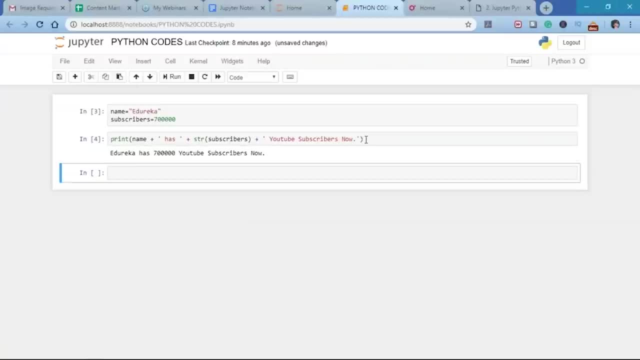 changed from one to three and if i rerun this, the cell number will change from two to four. so what jupyter does is keeps a track of the latest version of each cell. so, similarly, if you were to close the browser tab, refresh the display in the home tab. you will find a new item. we 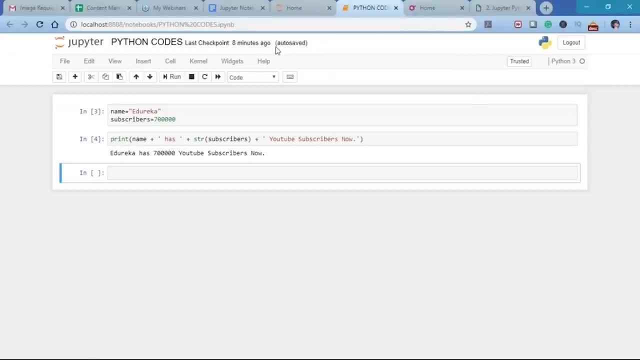 created, which is the python code. yeah, notebook saved, auto saved. as you can see here in the bracket it has auto saved. so if you close this in the home button, you can see here we have python codes. so, as you can see, if we click it it opens the same. 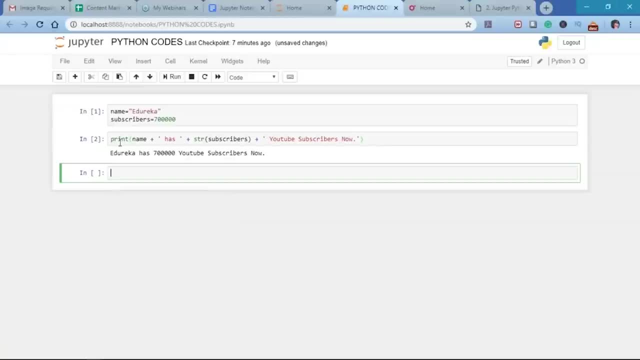 trending Technologies. So note that Jupiter color codes your python, just as decent editor would, and we have empty braces to the left of each code block. So, as you can see here, if we execute the cell, the results are displayed in line. Now it's interesting that Jupiter keeps track of the output last generated. 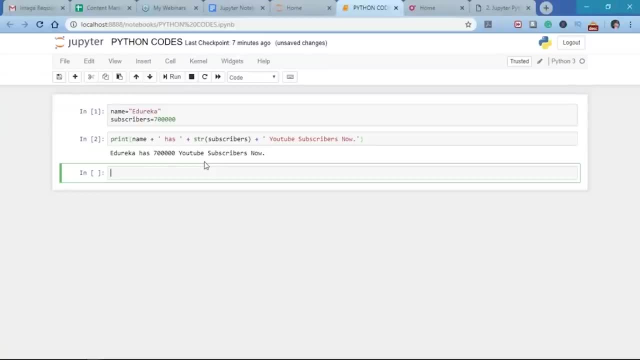 in the saved version of the file and is a safe checkpoints. Now, if you were to rerun your cells using the rerun or the run, all the output It would be generated and saved by autosave. Now the cell number is incremented and, as you can see, if I rerun this, you see 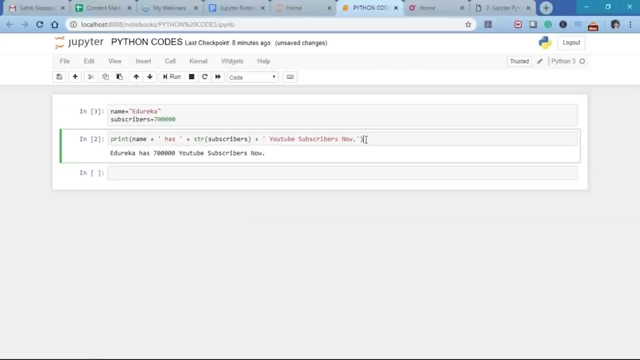 the cell number change from 1 to 3, and if I rerun this, the cell number will change from 2 to 4.. So what Jupiter does is keeps a track of the latest version of each cell. So, similarly, if you were to close the browser tab, refresh the display in. 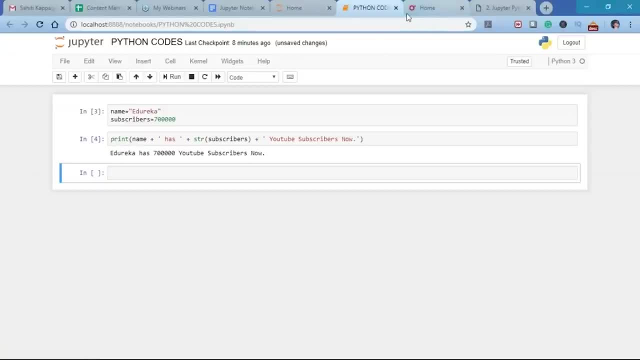 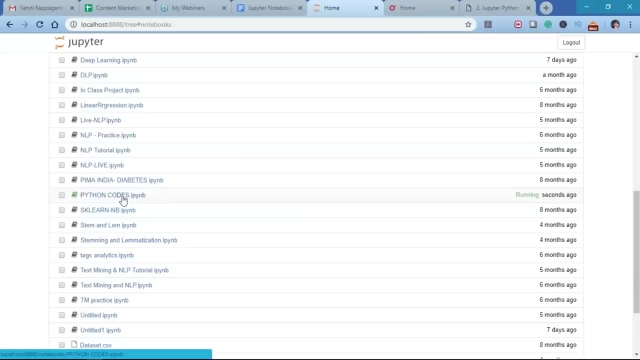 the home tab you will find a new item We created, which is the python code. Yeah, notebook saved, autosaved. as you can see here in the bracket It has autosaved. So if you close this in the home button, you can see: here we have python. 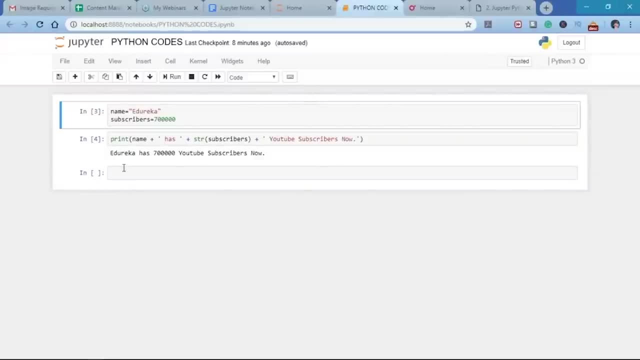 codes So, as you can see, if you click it it opens the same notebook It has. the previously displayed items will be always there, showing the output sweat that we generated in the last run. Now that we have seen how python works in Jupiter, including the underlying- 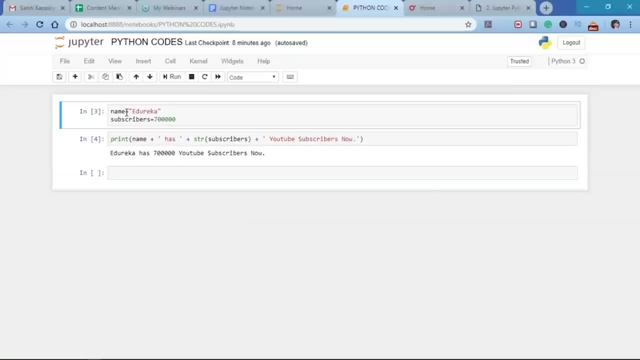 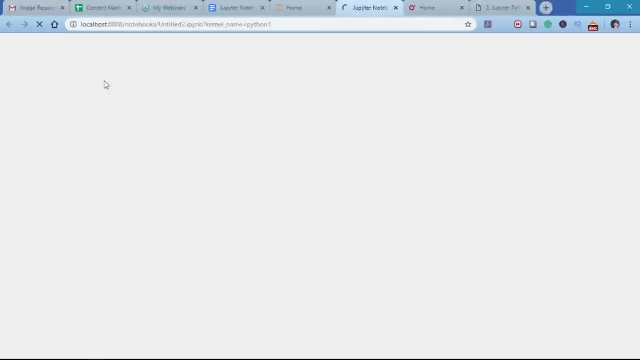 encoding. then how does python access a last data set? or data set work in Jupiter? So let me create another new python notebook. So what I'm going to do is name this as pandas. So from here, what we'll do is read in large data set and compute some. 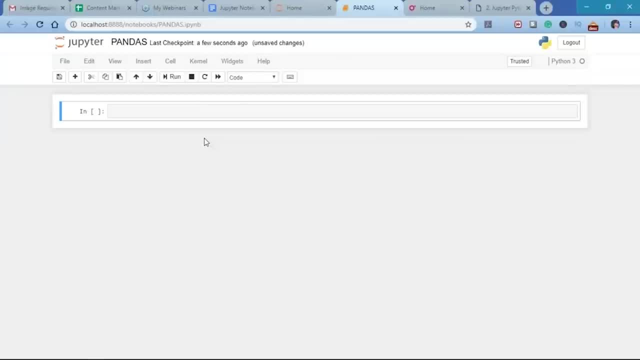 standard statistics of data. Now what we are interested in, and seeing how to use the pandas in Jupiter, how well the script performs and what information is stored in the metadata, especially if it's a large data set. So our python script accesses the iris data set here that's built into one. 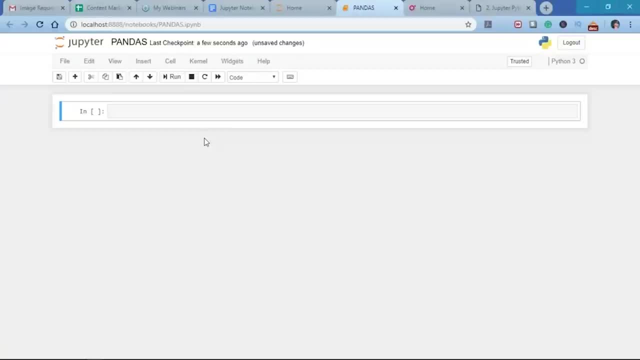 of the python packages. Now all we are looking into to do is to read in Slightly large number of items and calculate some basic operations on the data set. So first of all, what we need to do is, from sklearn, import the data set. 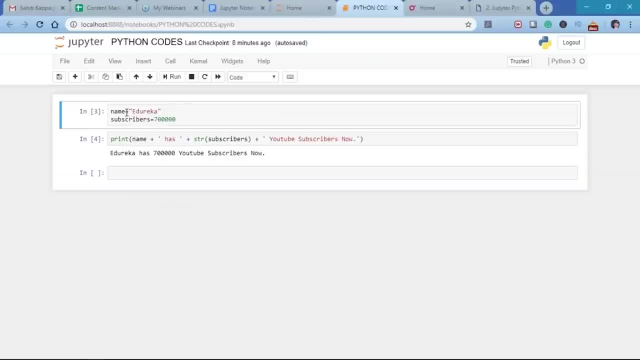 notebook it has. the previously displayed items will be always there, showing the outputs that we generated in the last run. now that we have seen how python works in jupyter, including the underlying encoding, then how does python access a last data set, or a data set work in jupyter? 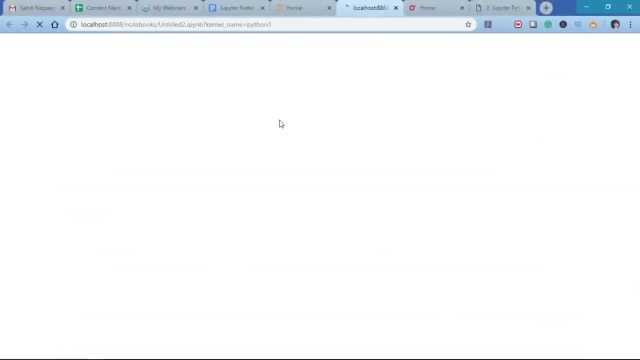 so let me create another new python notebook. so what i'm going to do is name this as pandas. so from here what we'll do is read in last data set and compute some standard statistics of data. now, what we are interested in, in seeing how to use the pandas in jupyter, how well the script. 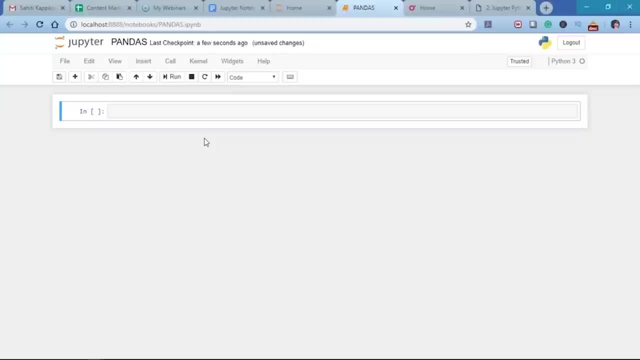 performs and what information is stored in the metadata, especially if it's a large data set. so our python script accesses the iris data set here. that's built into one of the python packages. now all we are looking into to do is to read in slightly large number of items and calculate some. 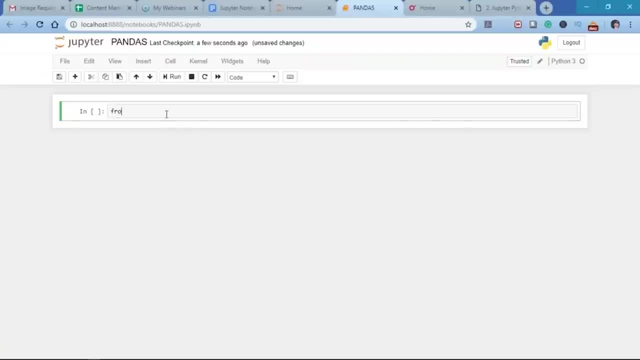 of the data set. so first of all, what we need to do is, from sklearn, import the data set. so sklearn is scikit-learn and it is another library of python. it contains a lot of data sets for machine learning and all the algorithms which are present for machine learning and the data sets. 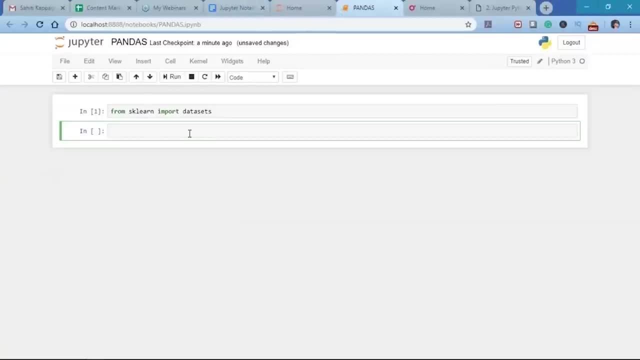 which are there. so. so our import was successful. so what we're going to do now is pull in the iris data. what we're going to do is: iris underscore data set equals data set dot load underscore iris. now this should do, and i'm sorry it's data set start load. so 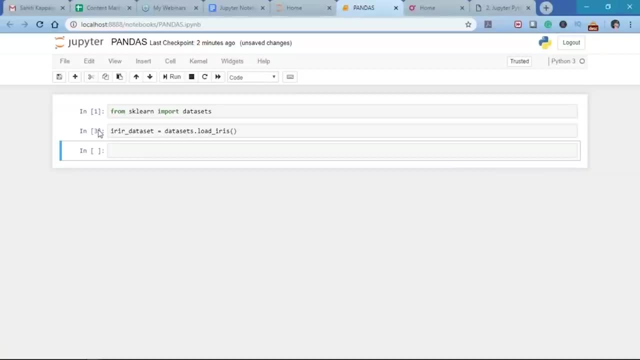 so, as you can see here, the number here is considered three now because in the second run we encountered an error. it was data set, not data set. so so, uh, what we're gonna do is grab the first two column of the data. so let's pretend x equals. if you press the tab, it automatically detects what. 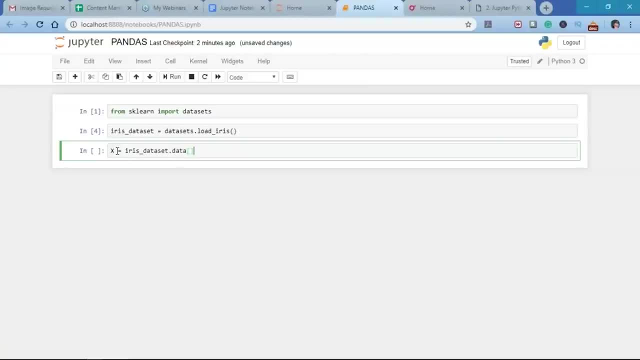 you're going to write as dot data set start data, and what we're going to do is take the first two rows comma. now to run it from your keyboard, all you need to do is press shift and enter. so next, what we're going to do is calculate some basic statistics. so what we're going to do is x underscore. 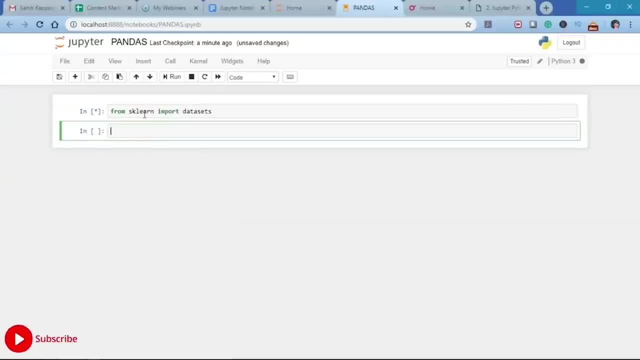 So sklearn is scikit-learn and it is another library of python. It contains a lot of data sets for machine learning and all the algorithms which are present for machine learning and the data sets which are there. So our import was successful. So what we're going to do now is pull in the iris data. 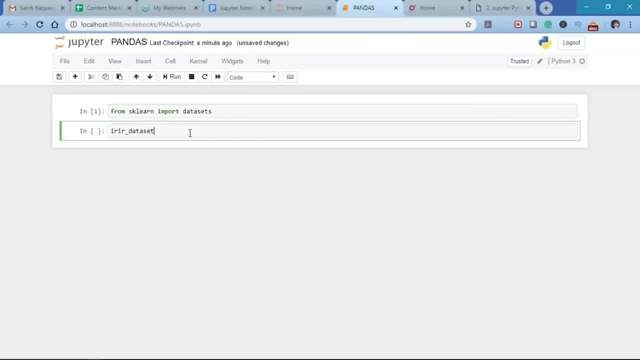 What we're going to do is iris underscore: Data set equals And the asset dot load underscore iris. Now, this should do and, I'm sorry, It's data set start load. So so, as you can see here, the number here is considered three now because 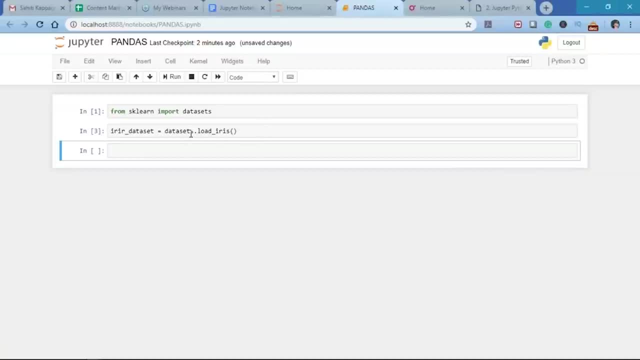 in the second run we encountered an error. It was data set, not data set. So so what we're going to do is grab the first two column of the data. So let's pretend x equals. If you press the tab, it automatically detects what you're going to write as. 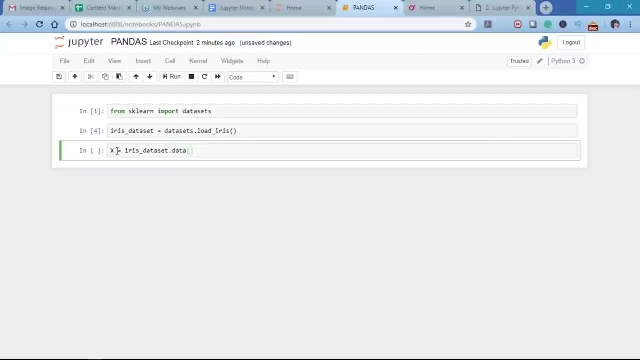 dot, data, set, start data, And what we're going to do is take the first two rows Comma not to run it from your keyboard. All you need to do is press shift and enter. So next, what we're going to do is calculate some basic statistics. 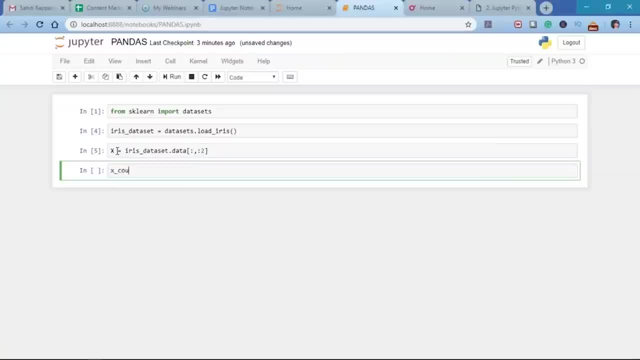 So what we're going to do is x underscore count equals x. We're going to use the length function and said that we're going to use x dot Flat. Similarly, we're going to see x min and x Max and the mean, our display, our. 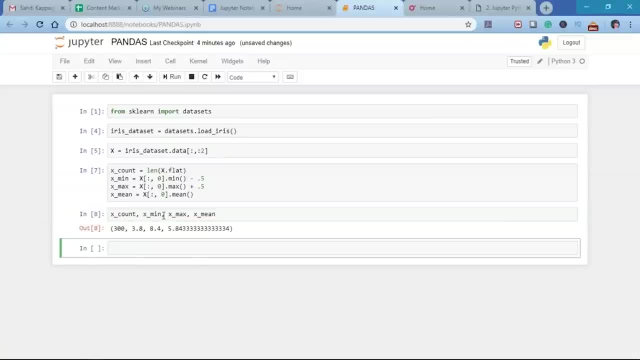 results. What we're going to do is to display the results now. So so, as you can see, the count is 300, the minimum value is 3.8.. The maximum, what is 8.4 and the mean is 5.8 for 333.. 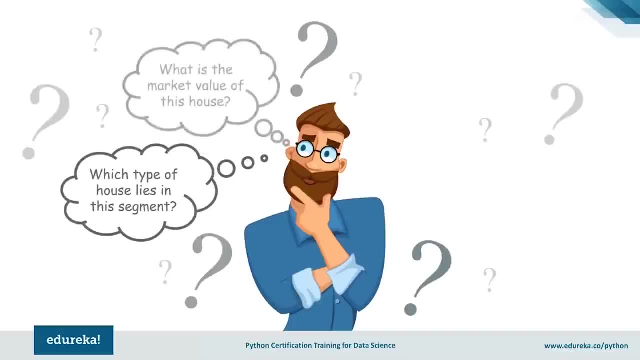 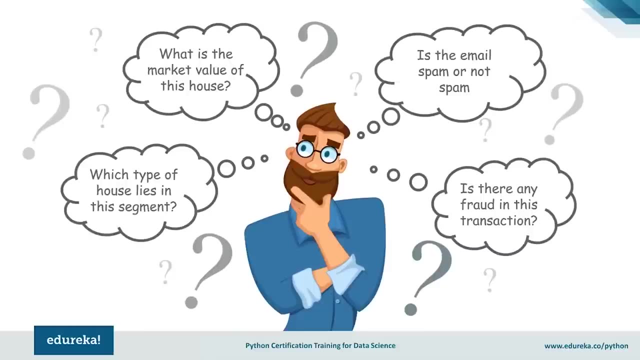 Let me connect you to the real life and tell you what all are the things which you can easily do using the concepts of machine learning, So you can easily get answer to the questions like which types of house lies in this segment or what is the market value of this house. 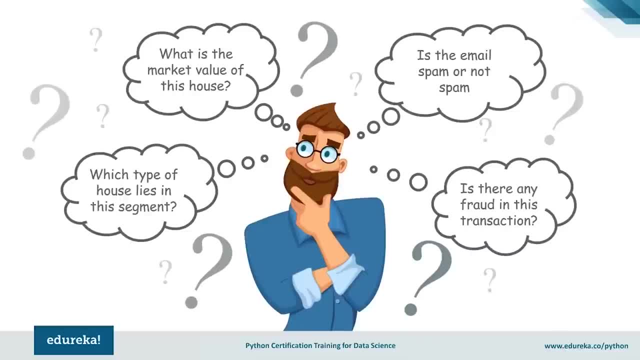 or is this a male, a spam or not a spam? Is there any fraud? Well, these are some of the question you could ask to the machine, but for getting an answer to these you need some algorithm. the machine need to train on the basis of some algorithm. 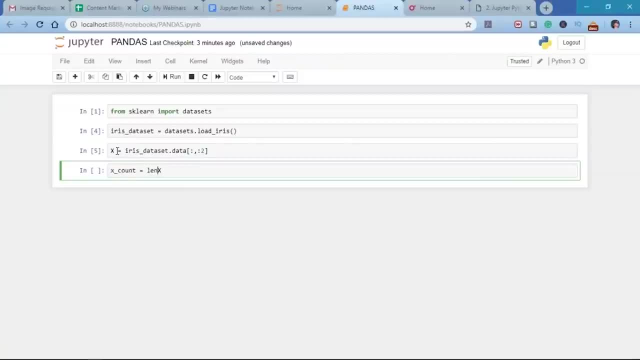 count equals x. we're going to use the length function and say that we're going to use xflat. similarly, we're going to see xflat, x min and x max and the mean. now to display our results. what we're going to do is to display the. 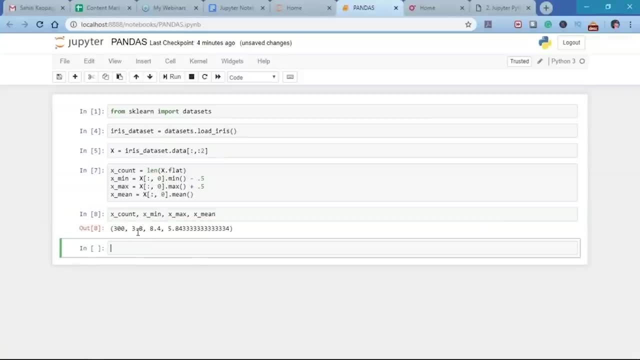 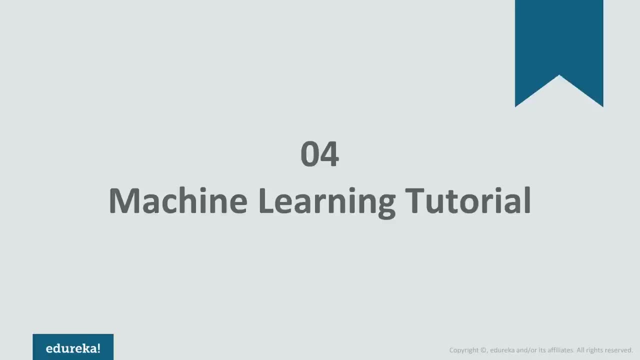 results now. so so, as you can see, the count is 300, the minimum value is 3.8, the maximum value is 8.4 and the mean is 5.84333. so let me connect you to the real life and tell you what all are the things. 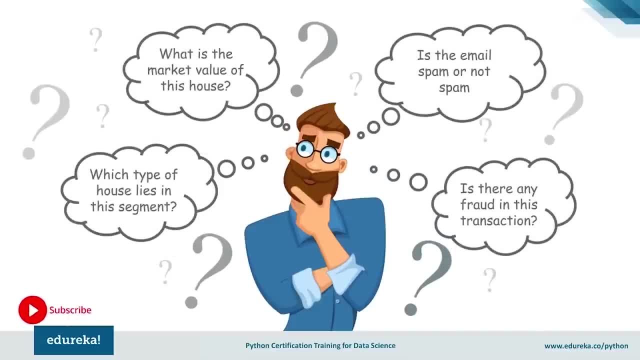 which you can easily do using the concepts of machine learning, so you can easily get answer to the questions like: what are the things that you can easily do using the concepts of machine learning, which types of house lies in this segment, or what is the market value of this house, or is this a male? 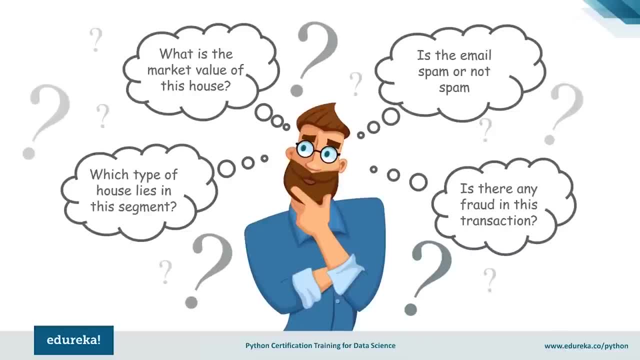 a spam or not a spam? is there any fraud? well, these are some of the question you could ask to the machine, but for getting an answer to these, you need some algorithm. the machine need to train on the basis of some algorithm. okay, but how will you decide which algorithm to choose and when? okay, so. 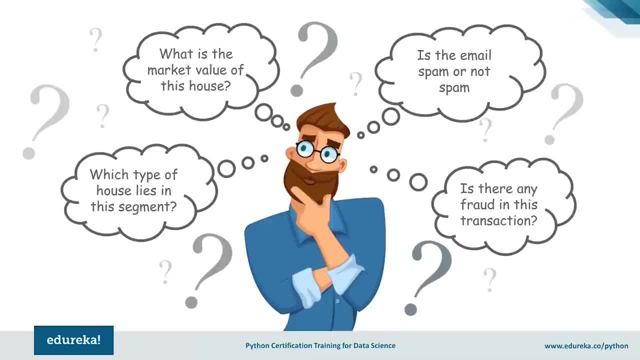 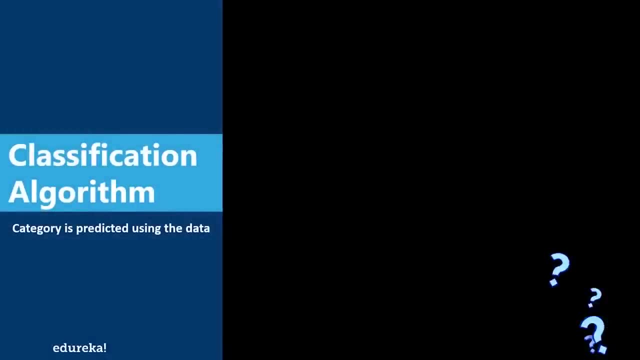 the best option for us is to explore them one by one. so the first is classification algorithm, where the category is predicted. you can use the classification algorithm and then you can use the data. if you have some question like is this person a male or a female, or is this male a spam or not, a 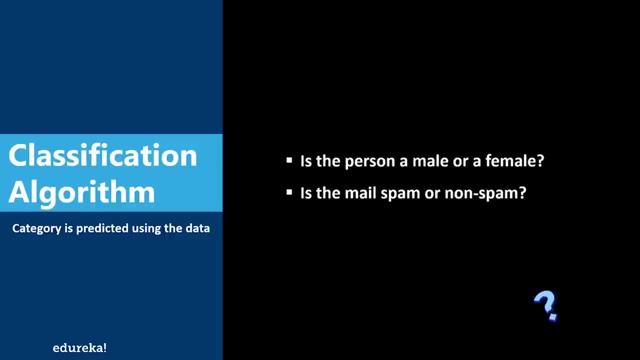 spam, then these category of question would fall under the classification algorithm. classification is a supervised learning approach in which the computer program learns from the input given to it and then uses this learning to classify new observation. some examples of classification problems are speech organization, handwriting organization, biometric identification document. 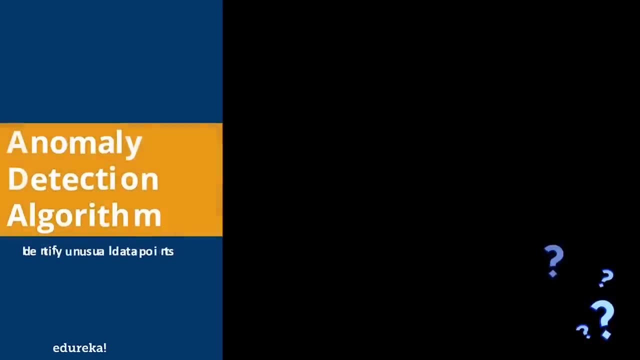 classification, etc. so next is the anomaly detection algorithm, where you identify the unusual data point. so what is anomaly detection? well, it's a technique that is used to identify unusual pattern that does not conform to expected behavior, or you can say the outliers. it has many application in business. 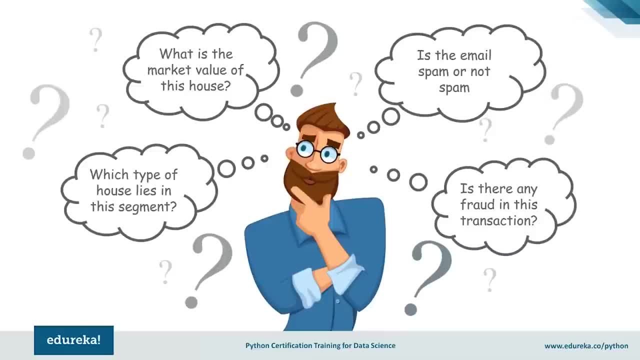 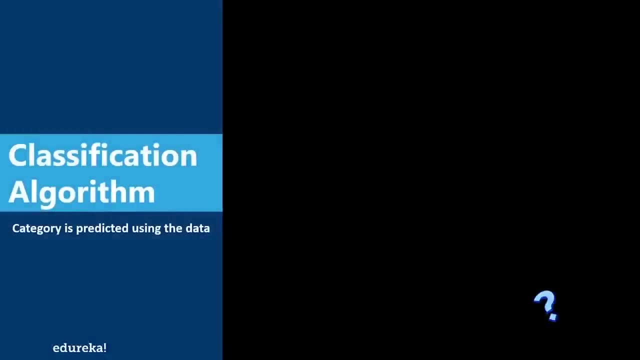 Okay, but how will you decide which algorithm to choose and when? Okay, so the best option for us is to explore them one by one. So the first is classification Algorithm, where the category is predicted using the data. If you have some question like: is this person a male or a female? 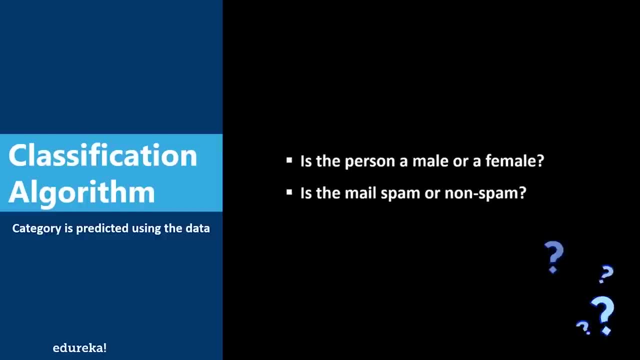 or is this male a spam or not a spam? then these category of question would fall under the classification algorithm. classification is a supervised learning approach in which the computer program learns from the input given to it and then uses this learning to classify new observation. Some examples of classification problems are speech organization. 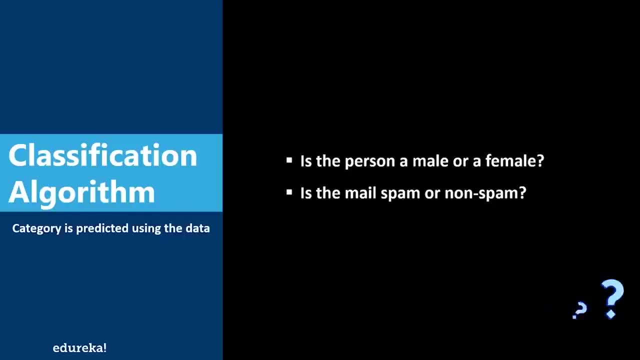 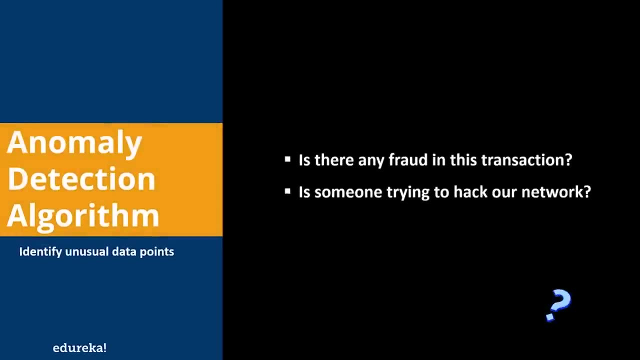 handwriting organization, biometric identity, Document classification, Etc. So next is the anomaly detection algorithm, where you identify the unusual data point. So what is anomaly detection? Well, it's a technique that is used to identify unusual pattern that did not confirm to expected behavior. or you can say the 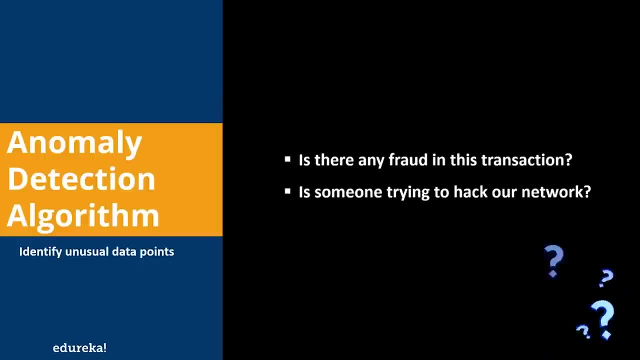 outliers. it has many application in business, like intrusion detection, like identifying strange patterns in the network traffic that could signal a hack, or system health monitoring that is spotting a deadly tumor in the MRI Scan. or you can even use it for fraud detection, credit card transaction or to deal with fault detection in operating environment. 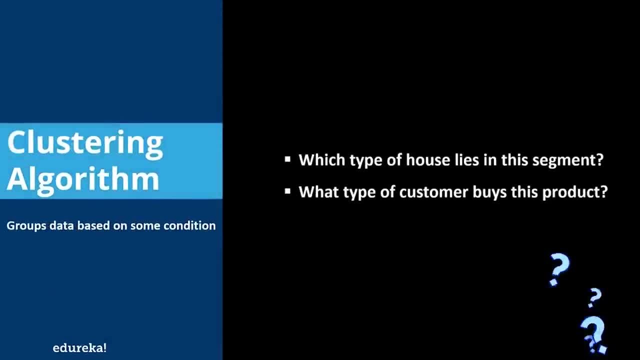 So next comes the clustering algorithm, and you can use this clustering algorithm to group the data based on some similar condition. Now you can get answer to which type of houses lies in this segment or what type of customer buys this product. the clustering is a task of dividing the population or data points into a number of groups. 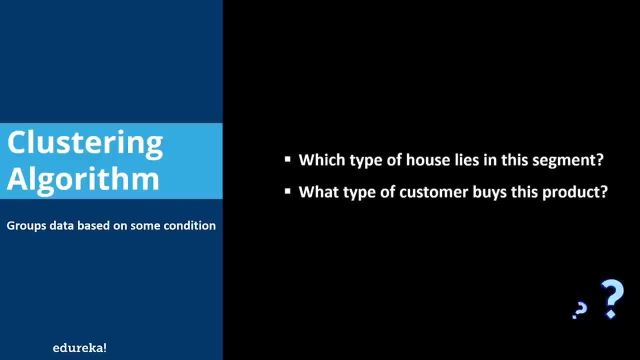 such that the data point and the same groups are more similar to other data points in the same group than those in the other groups. and simple words. The aim is to segregate groups with similar trait and assign them into cluster. Now this clustering is a task of dividing the population or data. 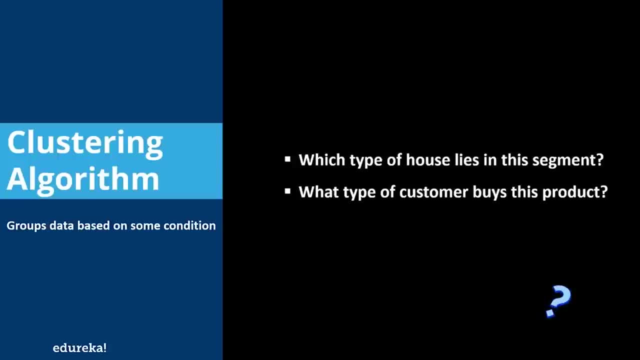 points into a number of groups, such that the data points in the X group is more similar to the other data points in the same group rather than those in the other group. In other words, the aim is to segregate the groups with similar traits and assign them into different clusters. 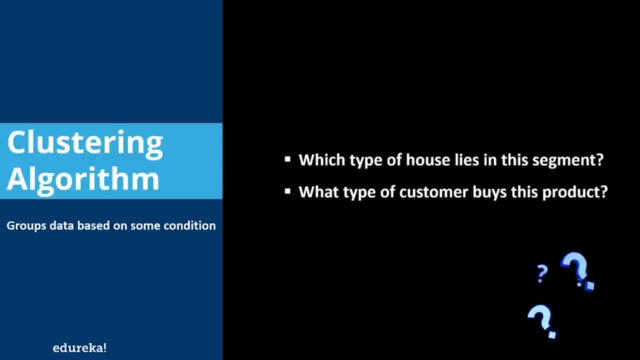 Let's understand this with an example. Suppose You're the head of a rental store and you wish to understand the preference of your customer to scale up your business. So is it possible for you to look at the detail of each customer and design a unique business strategy for each of them? definitely, 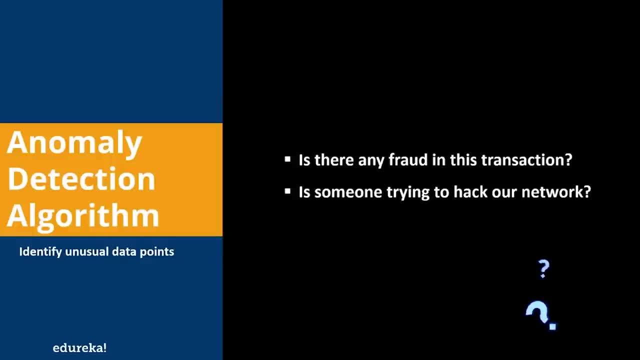 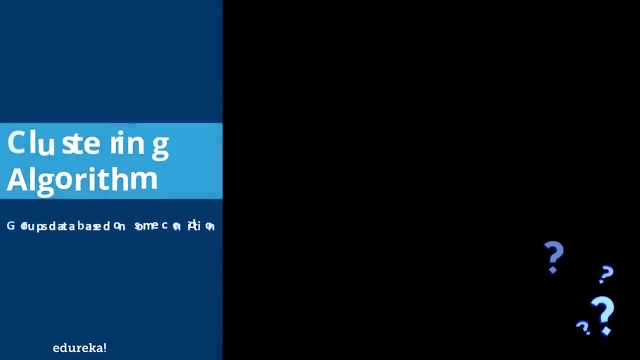 like intrusion detection, like identifying strange patterns in the network traffic that could signal a hack, or system health monitoring that is spotting a deadly tumor in the mri scan. or you can also use the anomaly detection credit card transaction or to deal with fault detection in operating environment. so next comes the clustering algorithm and you can use this. 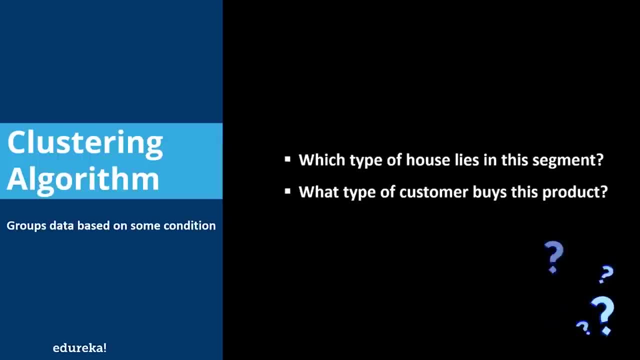 clustering algorithm to group the data based on some similar condition. now you can get answer to which type of houses lies in this segment or what type of customer buys this product. the clustering is a task of dividing the population or data points into number of groups, such that the data point and 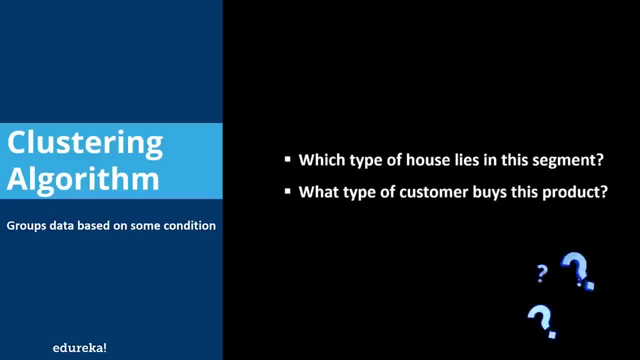 the same groups are more similar to other data points in the same group than those in the other. in simple words, the aim is to segregate groups with similar trait and assigning them into cluster. now this clustering is a task of dividing the population, or data points, into a number of 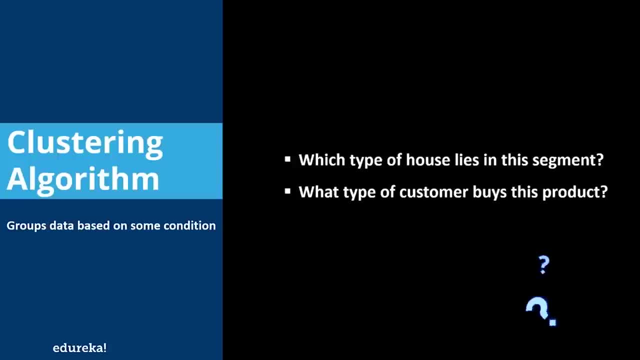 groups, such that the data points in the x group is more similar to the other data points in the same group rather than those in the other group. in other words, the aim is to segregate the groups with similar traits and assign them into different clusters. let's understand this with an example. 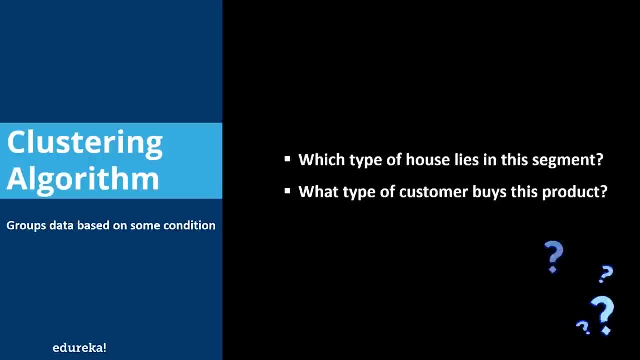 suppose you're the head of a rental store and you wish to understand the preference of your customer to scale up your business. So is it possible for you to look at the detail of each customer and design a unique business strategy for each of them? definitely not, right. 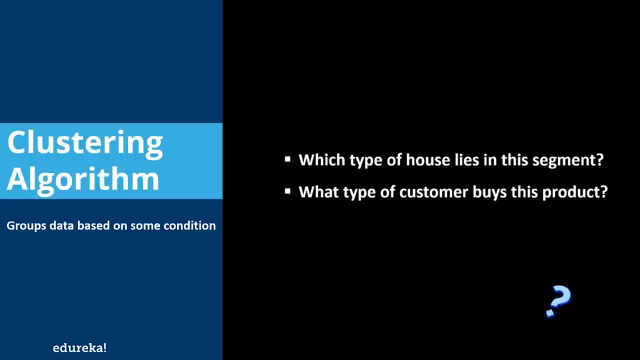 But what you can do is to cluster all your customer say into 10 different groups based on their purchasing habit, and you can use a separate strategy for customers in each of these 10 different groups, and this is what we call clustering. Next, we have regression algorithm. 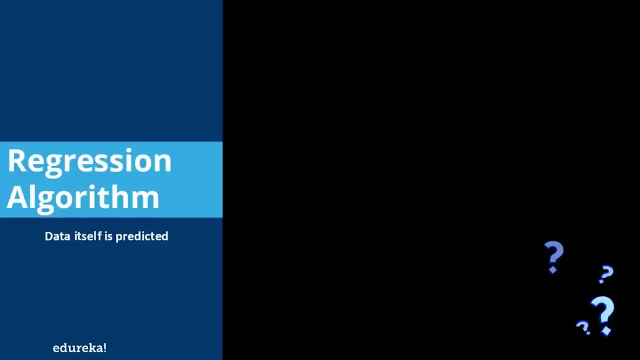 where the data itself is predicted. question you may ask to this type of model is like: what is the market value of this house, or is it going to rain tomorrow or not? So regression is one of the most important and broadly used machine learning and statistics tool. 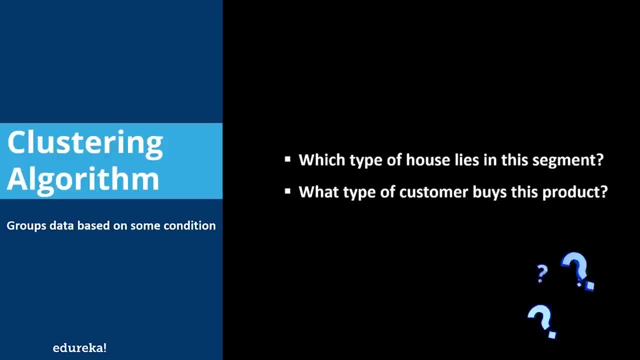 not right. But what you can do is to cluster all your customer say into 10 different groups based on their purchasing habit, and you can use a separate strategy for customers in each of these 10 different groups, and this is what we call clustering. Next, we have regression. 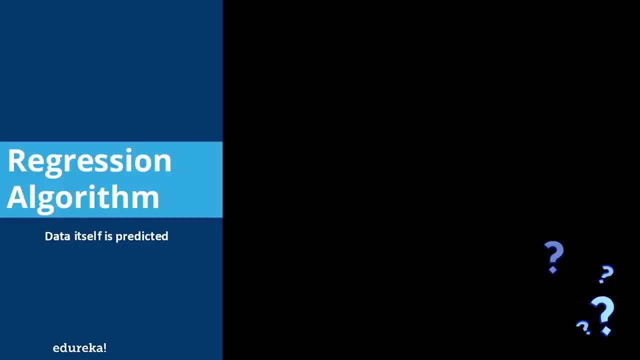 Algorithm where the data itself is predicted. question You may ask to this type of model is like: what is the market value of this house, or is it going to rain tomorrow or not? So regression is one of the most important and broadly used machine learning and statistics tool. 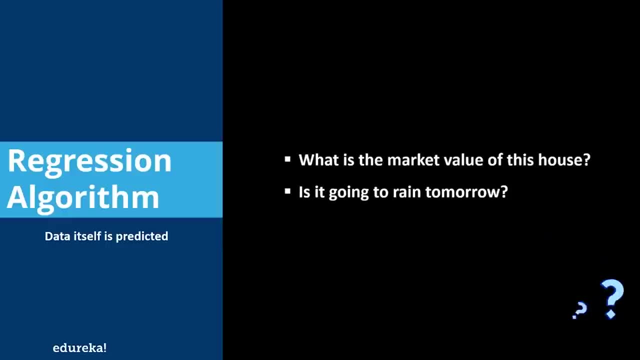 It allows you to make prediction from data by learning the relationship between the features of your data, and some observe continuous valued response. regression is used in a massive number of application. You know what stock prices prediction can be done using regression. Now you know about different machine learning algorithm. 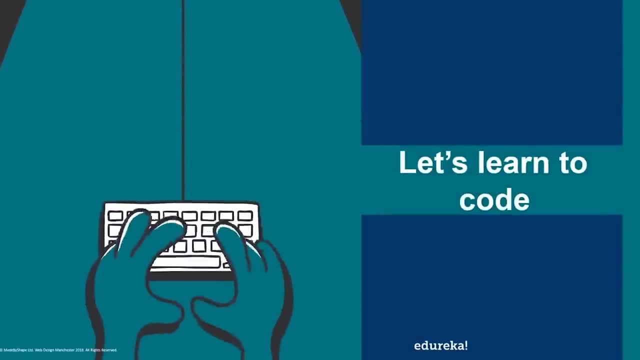 How will you decide which algorithm to choose and when? so let's cover this part using a demo. So in this demo part, what we'll do will create six different machine learning model and pick the best model and build the confidence such that it has the most reliable accuracy. 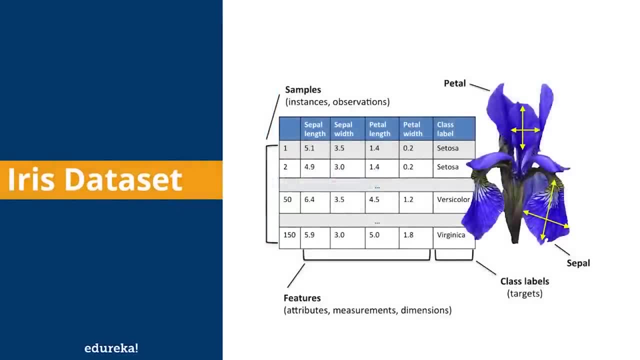 So for our demo part will be using the iris data set. This data set is quite, very famous and is considered one of the best small project to start with, you can consider this as a hello world data set for machine learning. So this data set consists of 150 observation of iris flower. 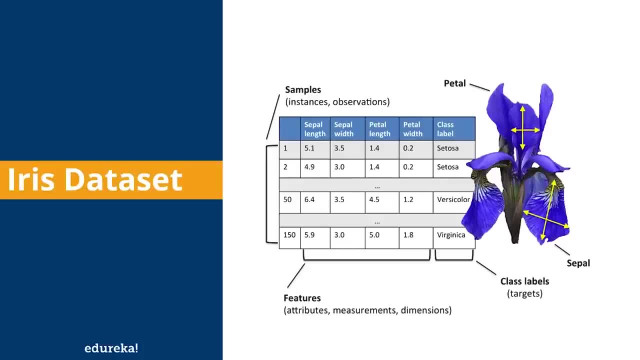 There are four columns of measurement of flowers in centimeters, the fifth column being the species of the flower observe. all the observed flowers belong to one of the three species of iris setosa, iris virginica and iris versicolor. Well, this is a good project because it is so well to 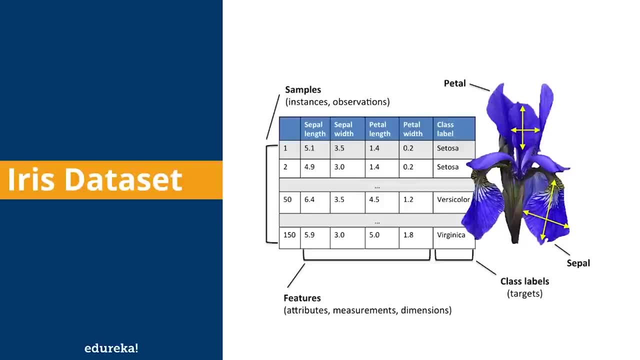 understand the attributes and numeric, So you have to figure out how to load and handle the data. It is a classification problem there. by allowing you to practice with perhaps an easier type of supervised learning algorithm. It has only four attributes and 150 rows, meaning it is very 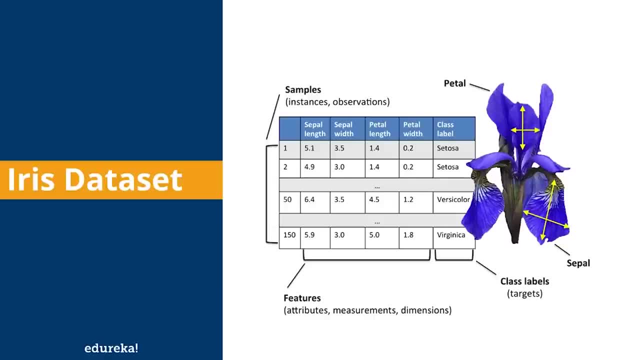 small and can easily fit into the memory, and even all of the numeric attributes are in same unit and the same scale means you do not require any special scaling or transformation to get started. So let's start coding, and as I told earlier for the demo part, 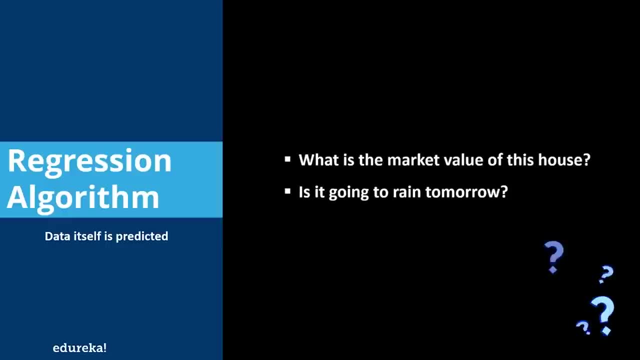 It allows you to make prediction from data by learning the relationship between the features of your data, and some observe continuous valued response. regression is used in a massive number of application. You know what stock prices prediction can be done using regression. now you know about different machine learning algorithm. 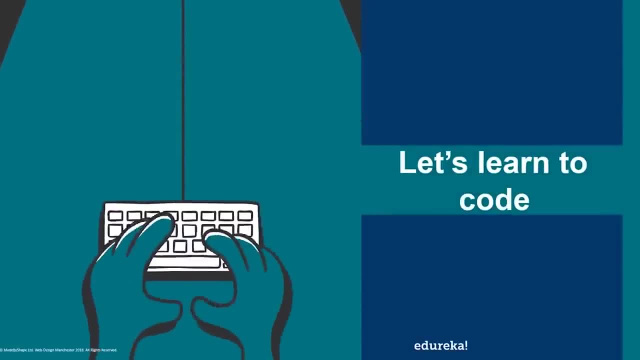 How will you decide which algorithm to choose and when? so let's cover this part using a demo. So in this demo part, what we'll do will create six different machine learning model and pick the best model and build the confidence such that it has the most reliable accuracy. 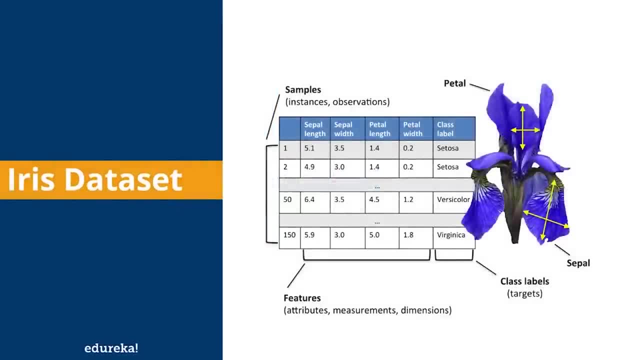 So for our demo part will be using the iris data set. This data set is quite, very famous and is considered one of the best small project to start with, you can consider this as a hello world data set for machine learning. So this data set consists of 150 observation of iris. 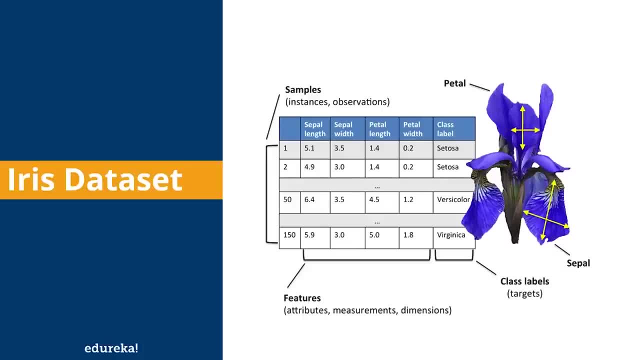 There are four columns of measurement of flowers in centimeters, the fifth column being the species of the flower observe. all the observed flowers belong to one of the three species of iris setosa, iris virginica and iris versicolor. Well, this is a good project. 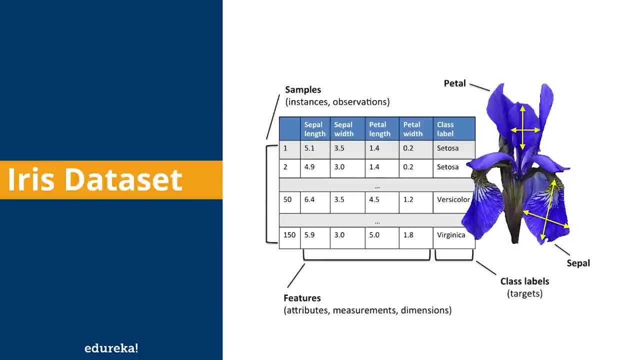 because it is so well to understand the attributes and numeric, so you have to figure out how to load and handle the data. It is a classification problem there, by allowing you to practice with perhaps an easier type of supervised learning algorithm. It has only four attributes. 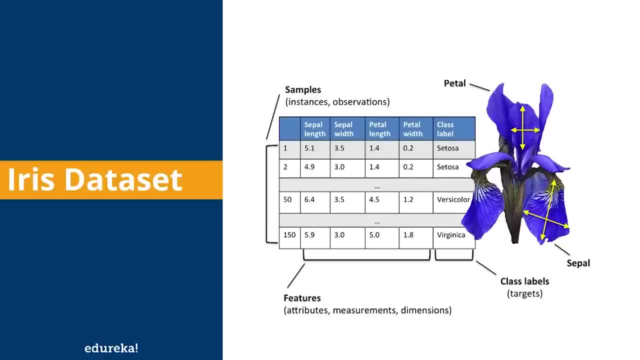 and 150 rows, meaning it is very small and can easily fit into the memory. and even all of the numeric attributes are in same unit and the same scale. It means you do not require any special scaling or transformation to get started. So let's start coding. 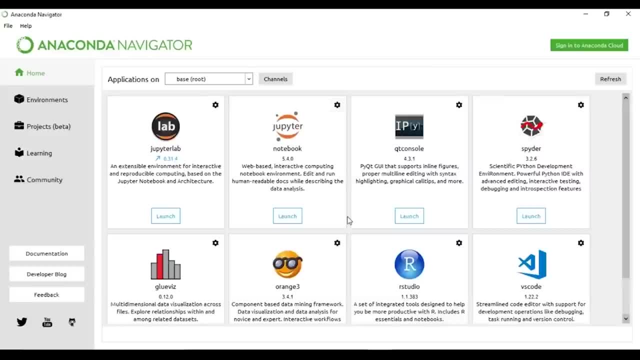 and, as I told earlier, for the demo part, I'll be using anaconda with python 3.0 install on it. So when you install anaconda, how your Navigator would look like. so there's my home page of my anaconda Navigator. on this: 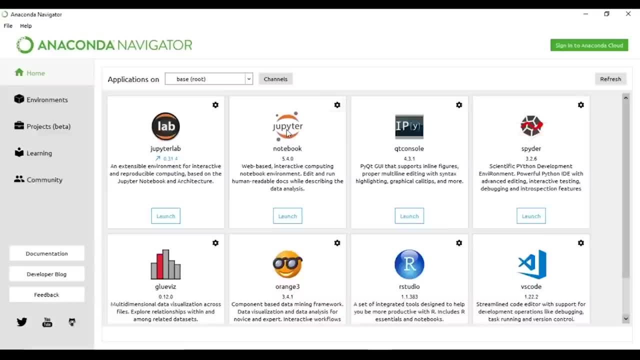 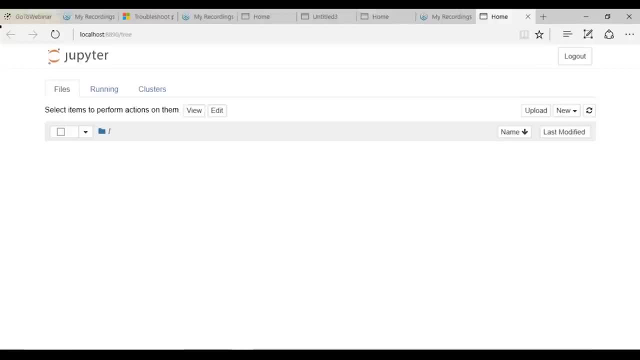 I'll be using the Jupiter notebook, which is a web-based interactive computing notebook environment which will help me to write and execute my python codes on it. So let's hit the launch button and execute our Jupiter notebook. So as you can see that my Jupiter notebook is starting. 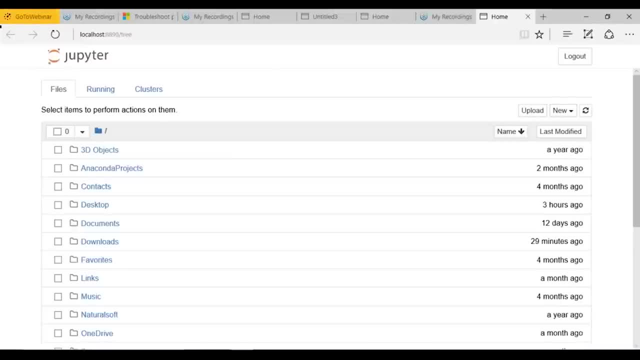 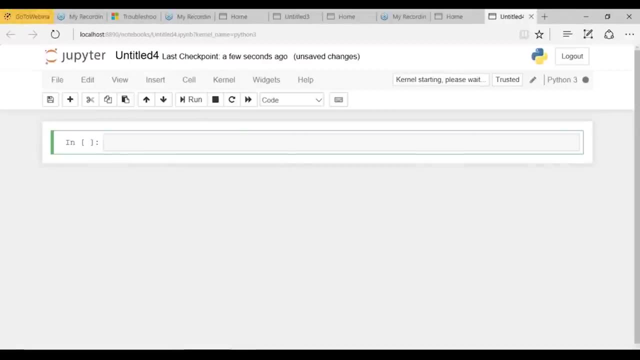 on localhost 8890.. Okay, so there's my Jupiter notebook. what I'll do here, I'll select new notebook, python 3.. There's my environment where I can write and execute all my python codes on it. So let's start by checking the version of the libraries. 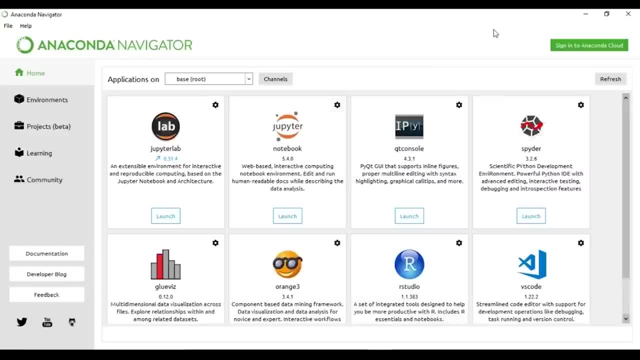 I'll be using anaconda with python 3.0 install on it. So when you install anaconda, how your Navigator would look like. so there's my home page of my anaconda Navigator. on this, I'll be using the Jupiter notebook, which is a web. 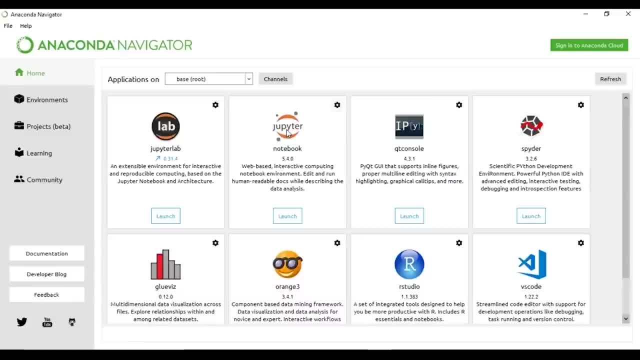 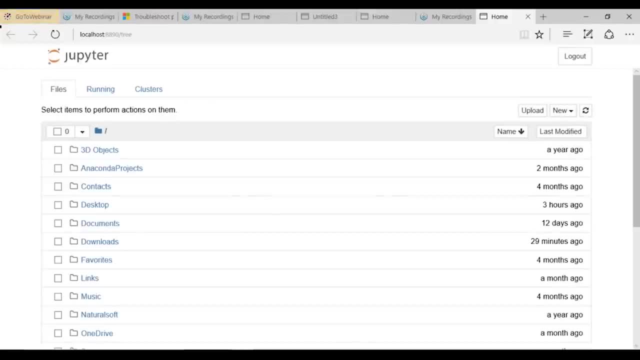 based interactive computing notebook environment which will help me to write and execute my python codes on it. So let's hit the launch button and execute our Jupiter notebook. So, as you can see that my Jupiter notebook is starting on localhost 8890.. Okay. 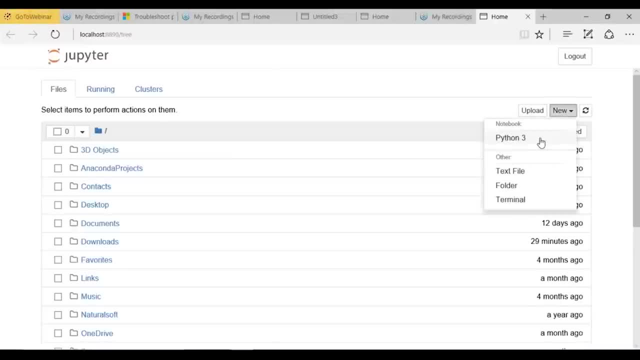 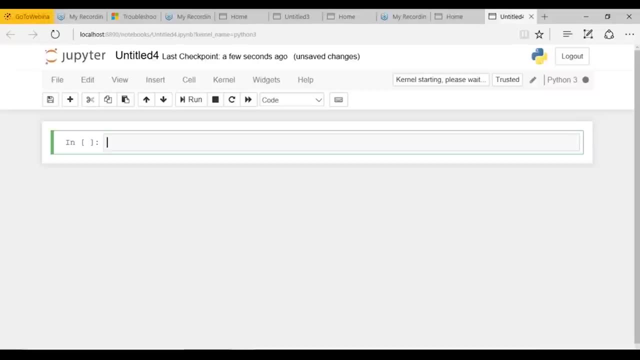 So there's my Jupiter notebook. what I'll do here? I'll select new notebook, python 3.. There's my environment, where I can write and execute all my python codes on it. So let's start by checking the version of the libraries in order to make this video short and more interactive. 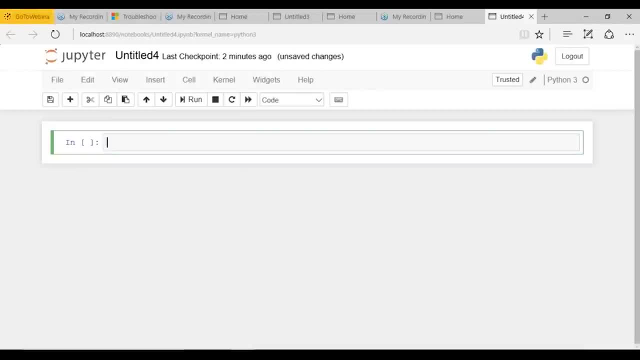 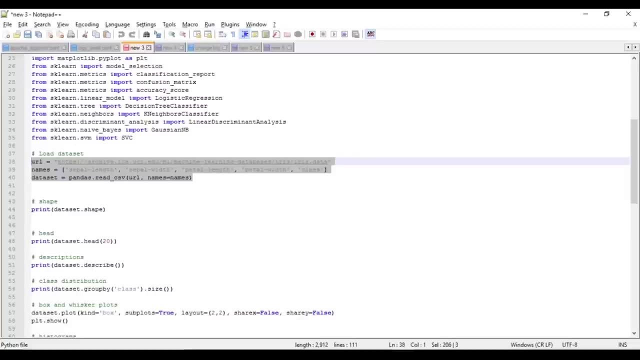 And more informative. I've already done the set of code, So let me just copy and paste it down. I'll explain you then one by one. So let's start by checking the version of the python libraries. Okay, so there's the code. 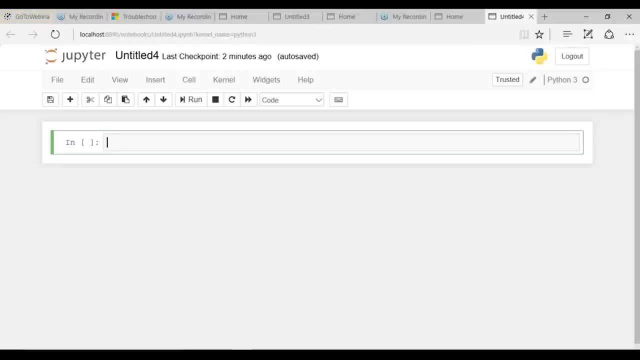 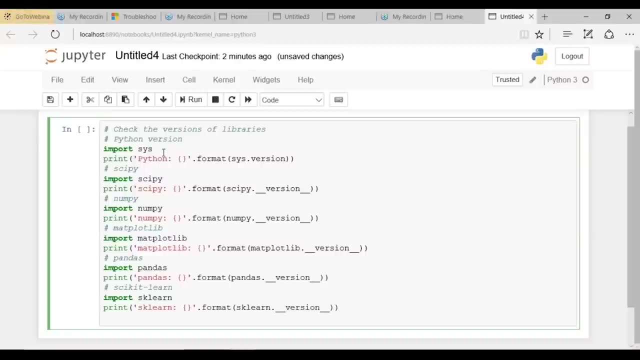 Let's just copy it copied and let's paste it, Okay? First Let me summarize things for you. What we are doing here: We are just checking the version of the different libraries, starting with python, will first check what version of python we are working on. then we'll check what are the version of. 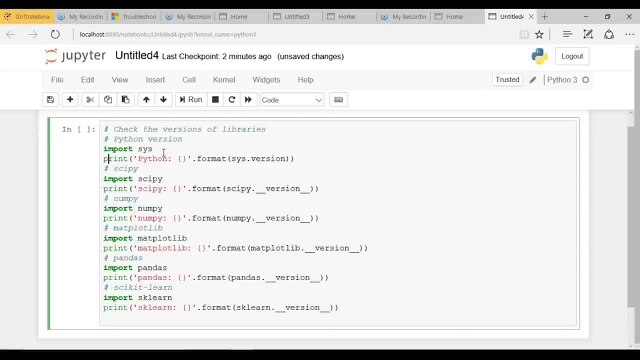 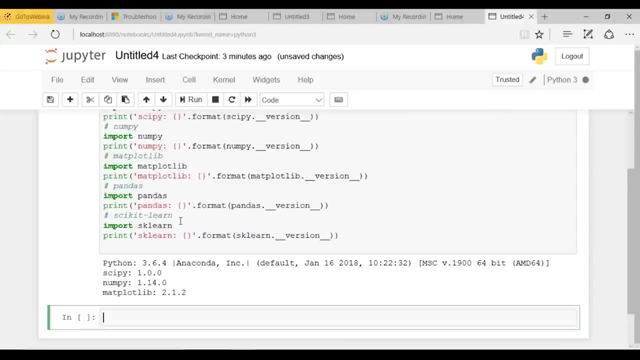 scipy we are using, then numpy, matplotlib, then Panda, then scikit-learn. Okay, so let's execute the run button and see what are the various version of libraries which we are using at the run. So we are working on python 3.6.4, scipy 1.0, numpy 1.14, matplotlib. 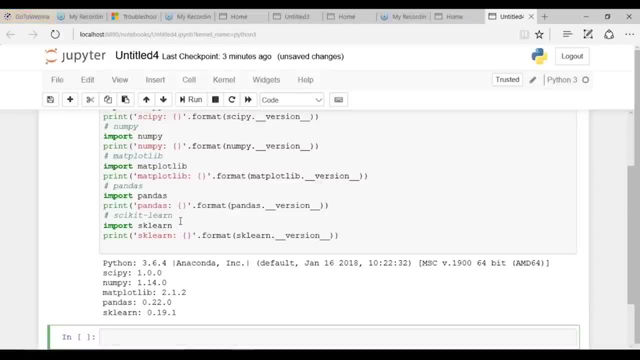 2.12, pandas 0.22 and scikit-learn of version 0.19.. Okay, So these are the version which I'm using. ideally, your version should be more recent or it should match, but don't worry if you love few versions behind, as the apis do not change so. 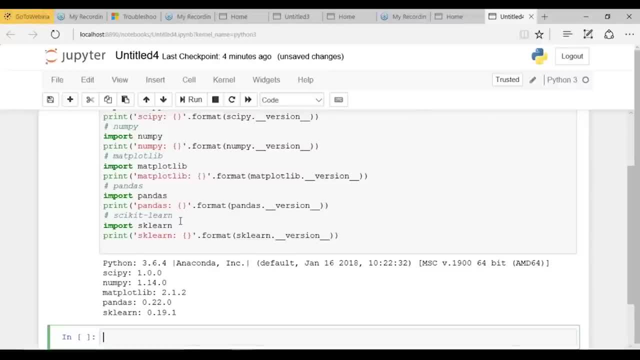 quickly everything in this tutorial. We'll very likely still work for you, Okay, but in case you are getting an error, stop and try to fix that error. in case you are unable to find the solution for the error, feel free to reach out edureka even after this. 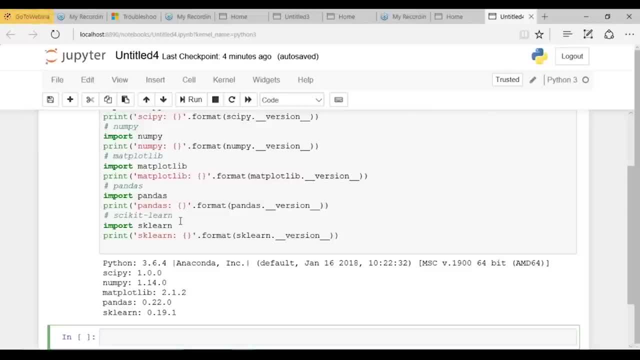 class. Let me tell you this: if you are not able to run the script properly, you will not be able to complete this tutorial. Okay, So whenever you get a doubt, reach out to edureka and just resolve it now. if everything is working smoothly, then now. 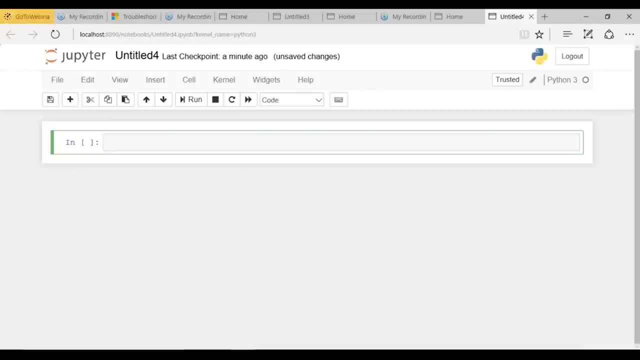 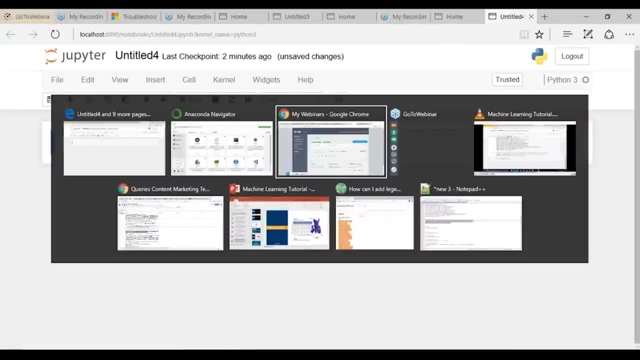 in order to make this video short and more interactive and more informative. I've already done The set of code, So let me just copy and paste it down. I'll explain you then, one by one. So let's start by checking the version of the python libraries. 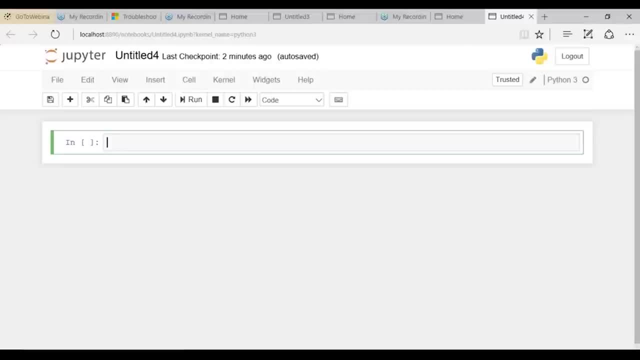 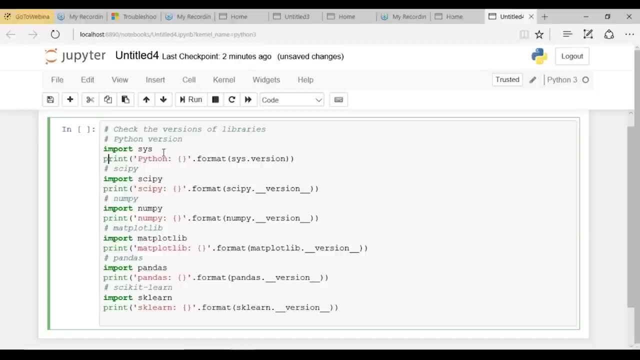 Okay, so there's the code, Let's just copy it copied and let's paste it. Okay, First Let me summarize things for you. What we are doing here: We are just checking the version of the different libraries, starting with python will first check what version of python. 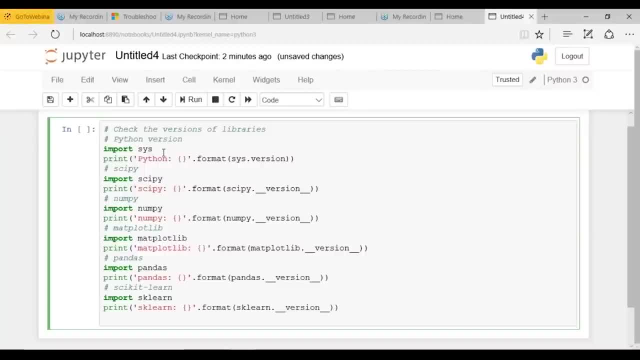 we are working on. then we'll check what are the version of scipy we are using, then numpy, matplotlib, then panda, then scikit-learn. Okay, So let's execute The run button and see what are the various version of libraries which we are using at the run. 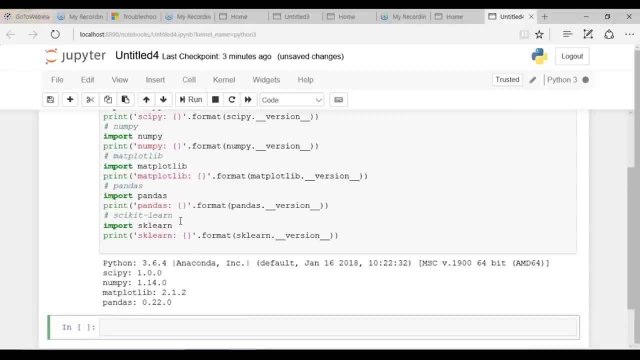 So we are working on python 3.6.. For scipy 1.0, numpy 1.14, matplotlib 2.12, pandas 0.22 and scikit-learn of version 0.19.. Okay, So these are the version which I'm using, ideally your version. 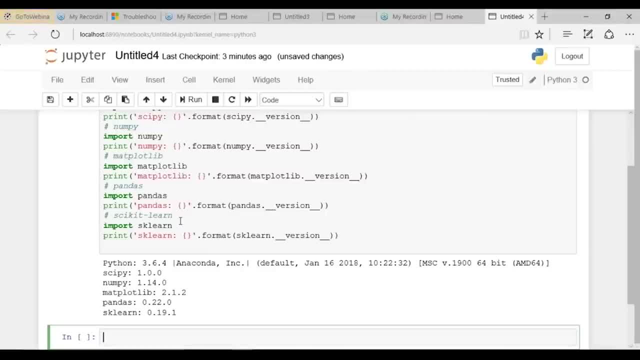 should be more recent or it should match. but don't worry if you love few versions behind, as the apis do not change so quickly. everything in this tutorial will very likely still work for you, Okay, But in case you are getting an error, stop and try to fix. 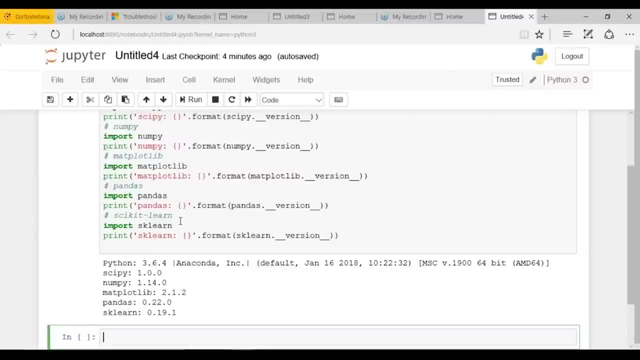 that error. in case you are unable to find the solution for the error, feel free to reach out edureka. even after this class, Let me tell you this: if you are not able to run the script properly, you will not be able to complete this tutorial. 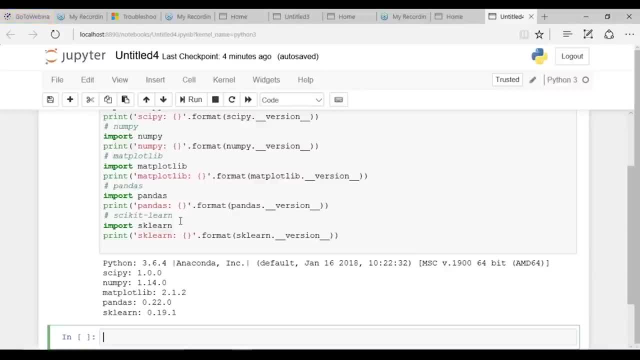 Okay. So whenever you get a doubt, reach out to edureka and just resolve it now. if everything is working smoothly, then now it's the time to load the data set. So, as I said, I'll be using the iris flower data set for this. 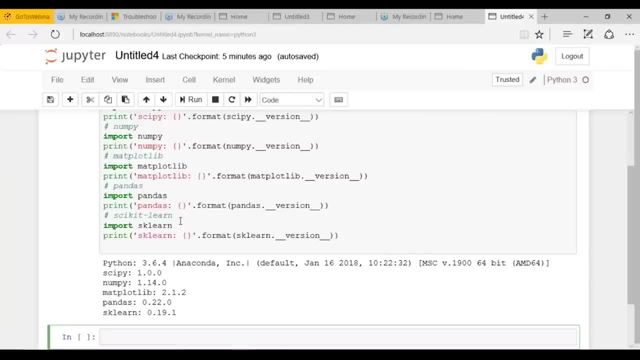 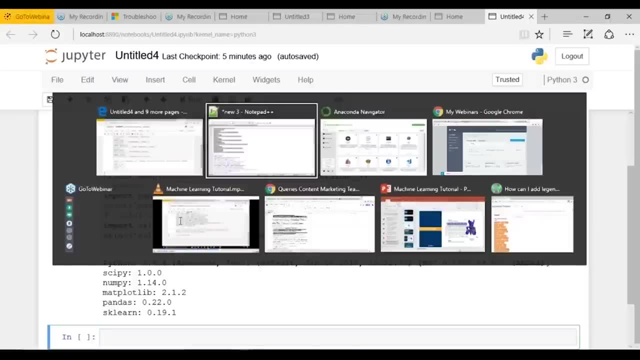 tutorial. but before loading the data set, let's import all the modules, function and the object which we are going to use in this tutorial same. I have already written the set of code, So let's just copy and paste them. Let's load all the libraries. 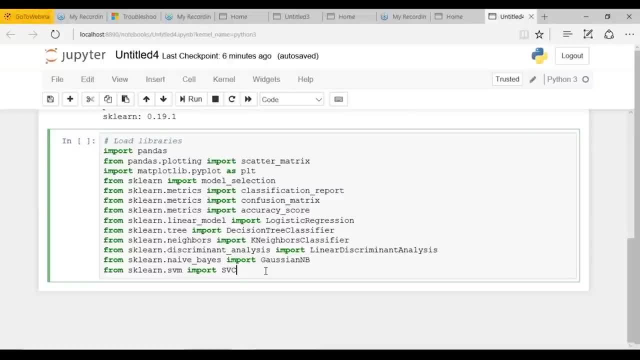 So these are the various libraries which will be using in our tutorial, So everything should work fine without an error. If you get an error, just stop. you need to work on your cyber environment before you continue any further. So I guess everything should work fine. 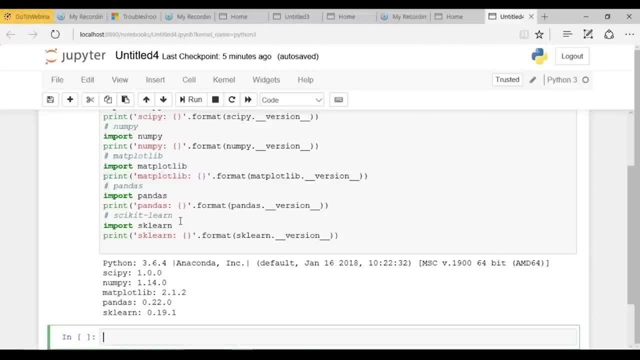 it's the time to load the data set. So, as I said, I'll be using the iris flower data set for this tutorial. But before loading the data set, let's import all the modules, function and the object which we are going to use in this. 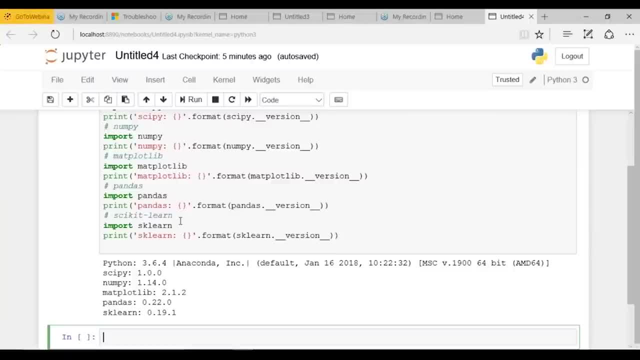 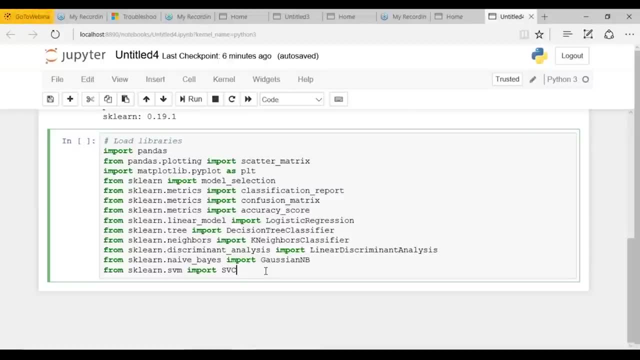 tutorial same. I've already written the set of codes, So let's just copy and paste them. Let's load all the libraries. So these are the various libraries which will be using in our tutorial. So everything should work fine without an error. 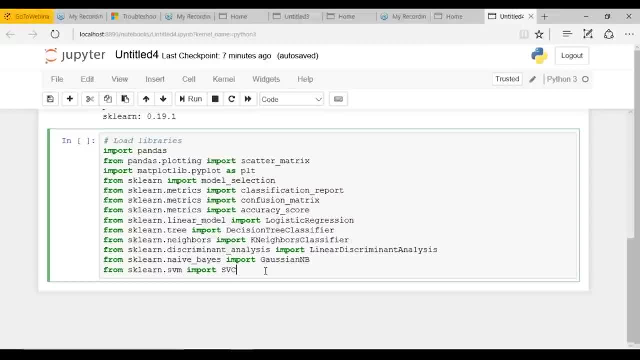 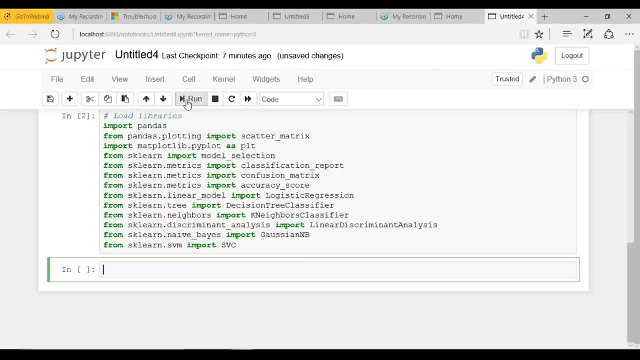 If you get an error, just stop. you need to work on your cyber environment before you continue any further, So I guess everything should work fine. Let's hit the run button and see: Okay, it worked. So let's now move ahead and load the data. we can load the. 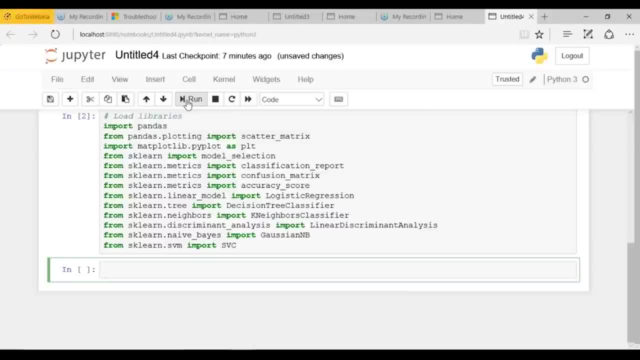 data direct from the UCI machine learning repository. First of all, let me tell you we are using Panda to load the data. Okay, So let's say my URL is this. so this is my URL for the UCI machine learning repository, from where I'll be downloading. 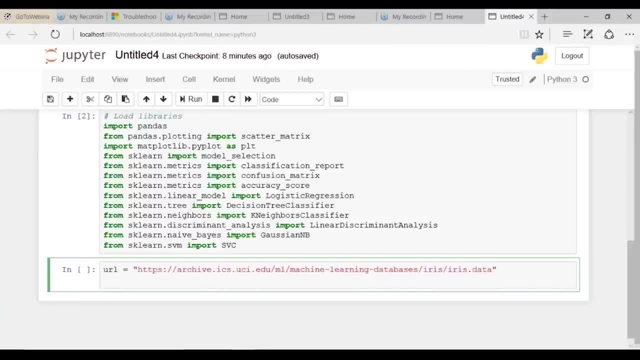 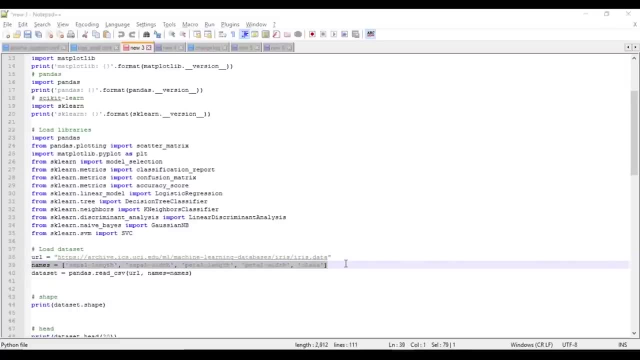 the data set. Okay, Now what I'll do. I'll specify the name of each column when loading the data. This will help me later to explore the data. Okay, so I'll just copy and paste it down. Okay, so I'm defining a variable name. 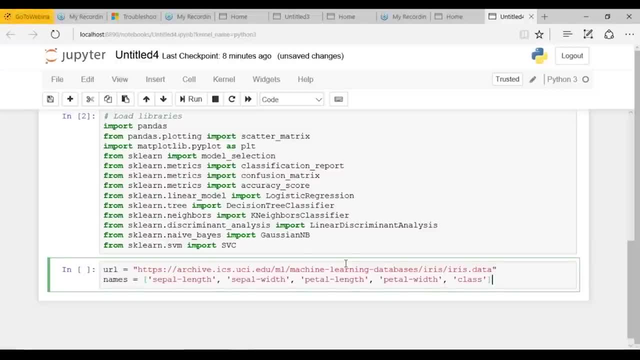 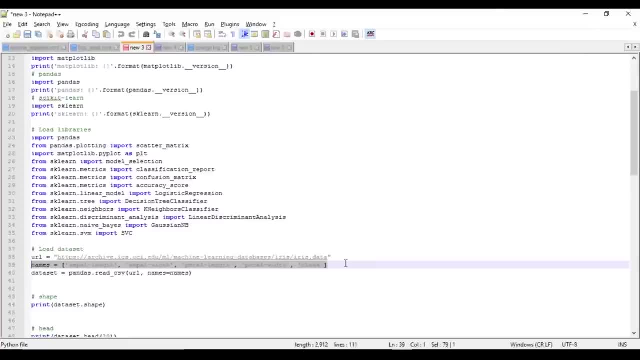 Names, which consists of various parameters, including separate separate petal and petal width and class. So these are just the name of column from the data set. Okay, Now let's define the data set. So data set equals Panda dot read underscore CSV inside that. 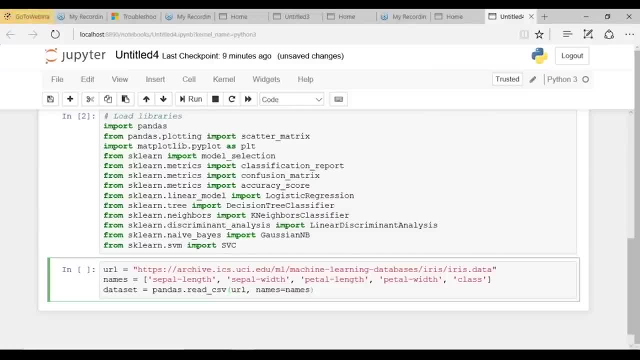 we are defining URL and the names- that is equal to name- as I already said, will be using Panda to load the data. All right, so we are using Panda dot read CSV. So we are reading the CSV file and, inside that, from where that CSV is coming from, the URL. 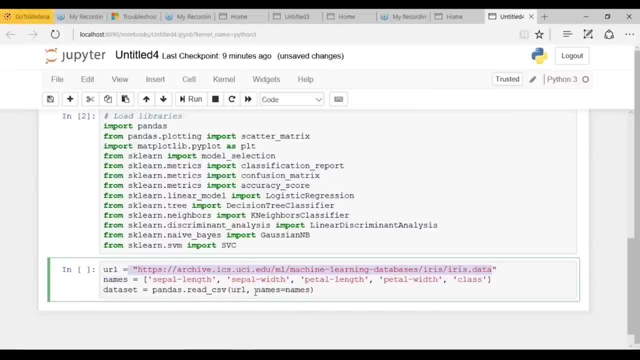 Which URL? so there's my URL. Okay, our name, sequel names: It's just specifying the names of that various columns in that particular CSV file. Okay, so let's move forward and execute it, So even our data set is loaded. in case you have some network, 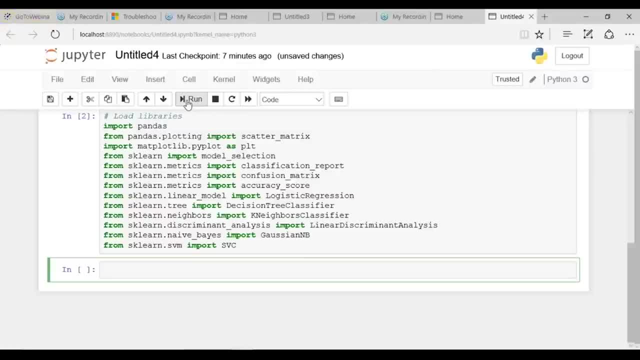 Let's hit the run button and see: Okay, it worked. So let's now move ahead and load the data. We can load the data direct from the UCI machine learning repository. First of all, let me tell you we are using Panda to load the. 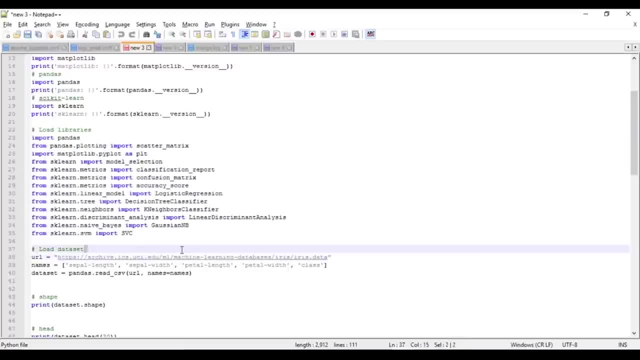 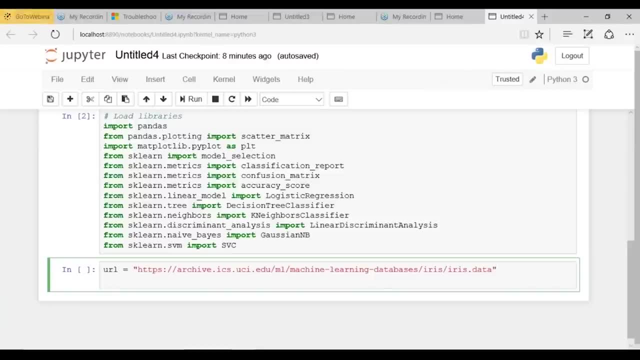 data. Okay, so let's say my URL is this. so this is my URL for the UCI machine learning repository, from where I'll be downloading the data set. Okay, Now what I do. I'll specify the name of each column when loading the data. 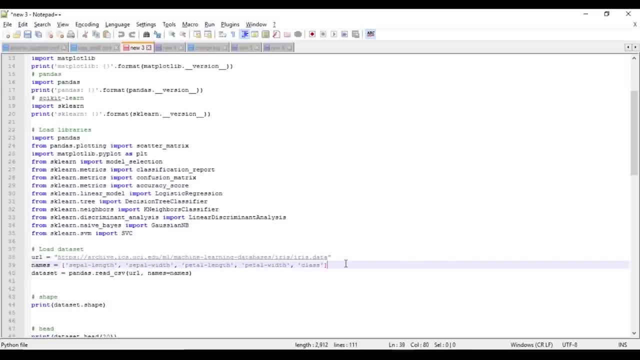 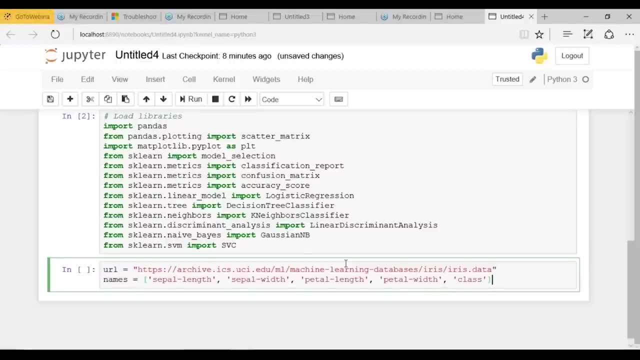 This will help me later to explore the data. Okay, so I'll just copy and paste it down. Okay, so I'm defining a variable names which consists of various parameters, including sepal and sepal with petal and petal with, and class. 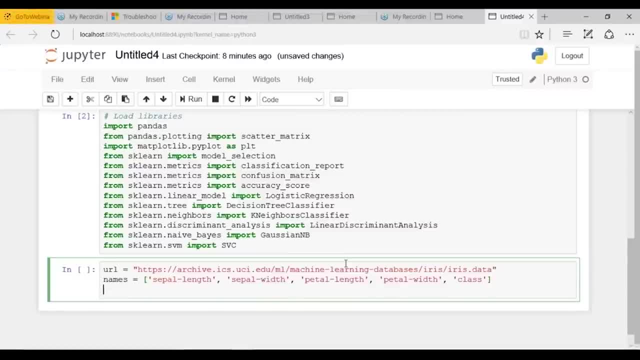 So these are just the name of column from the data set. Okay, Now let's define the data set. So data set equals Panda dot. read underscore CSV. inside that we are defining URL and the names- that is equal to name. As I already said, will be using Panda to load the data. 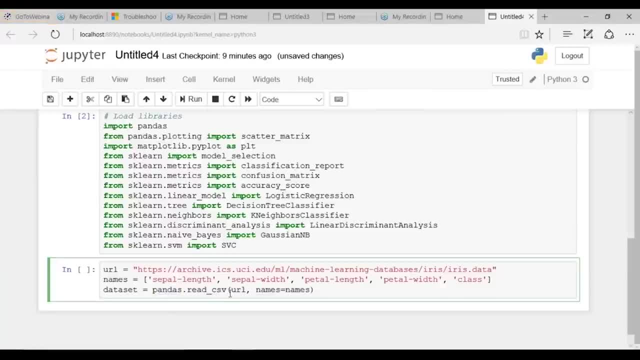 All right, so we are using Panda dot read CSV. So we are reading the CSV file and inside that, from where that CSV is coming from, the URL, which URL? So this is my URL. Okay, our name, sequel names. It's just specifying the names of that various columns in that. 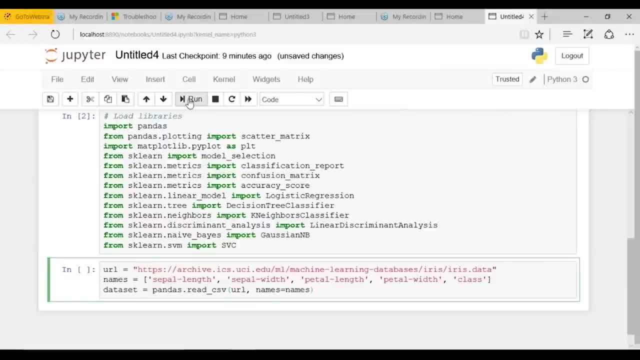 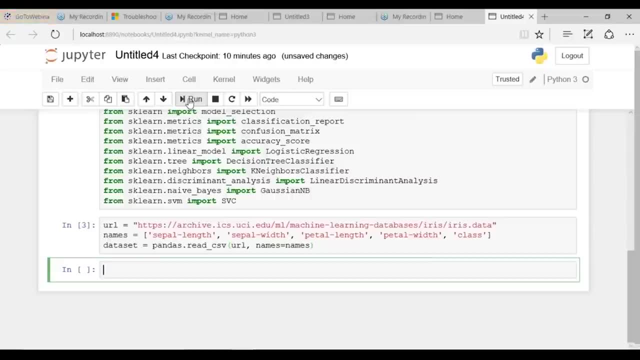 particular CSV file. Okay, So let's move forward and execute it. So even our data set is loaded. in case you have some network issues, Just go ahead and download the iris data file into your working directory and load it using the same method. 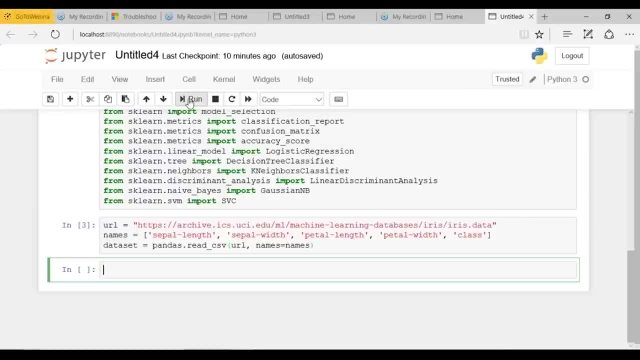 But, yeah, make sure that you change the URL to the local name, or else you might get an error. Okay, Yeah, data set is loaded, So let's move ahead and check out data set. Let's see how many columns or rows We have in our data set. 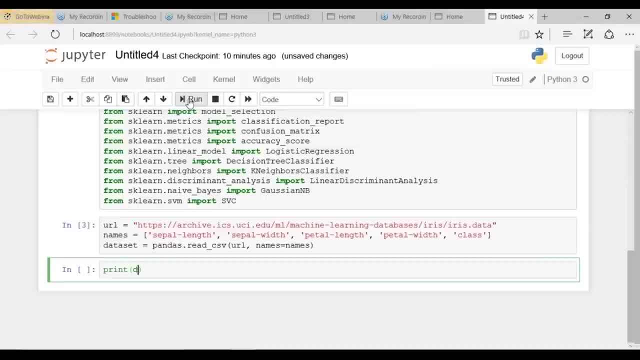 Okay, So let's print the number of rows and columns in our data set. So our data set is data set dot shape. what this will do, It will just give you the numbers of total number of rows and total number of column, or you can say the total number of. 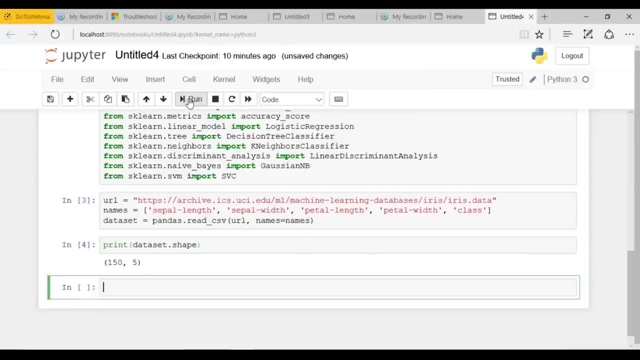 instances or attributes in your data set. fine, So print data set dot shape. What do you are getting? 150 and 5. so 150 is the total number of rows in your data set and 5 is the total number of columns. fine, So moving on ahead. 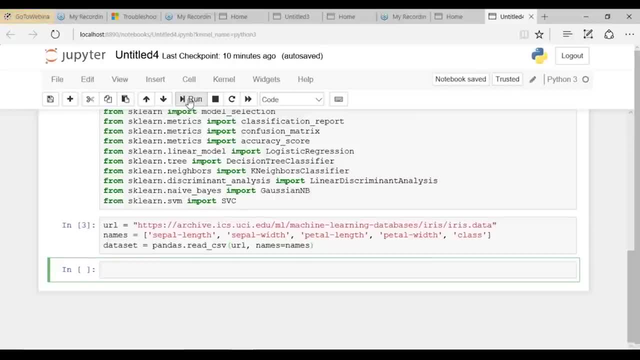 issues. Just go ahead and download the iris data file into your working directory and load it using the same method. But, yeah, make sure that you change the URL to the local name, or else you might get an error. Okay, Yeah, data set is loaded. 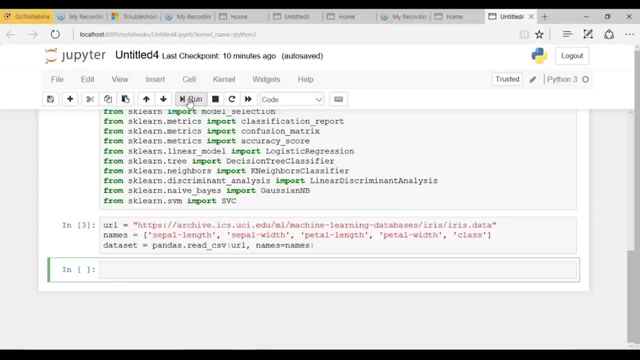 So let's move ahead and check out data set. Let's see How many columns or rows we have in our data set. Okay, so let's print the number of rows and columns in our data set. So our data set is data set dot shape. what this will do. 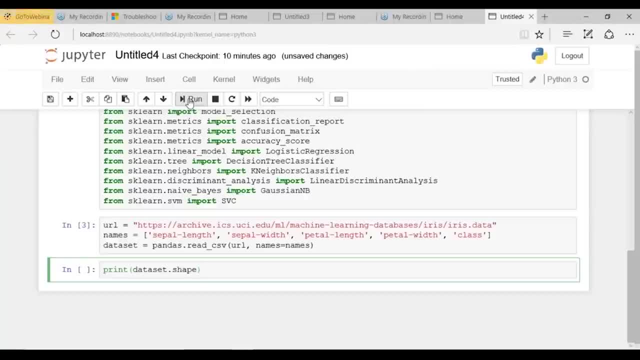 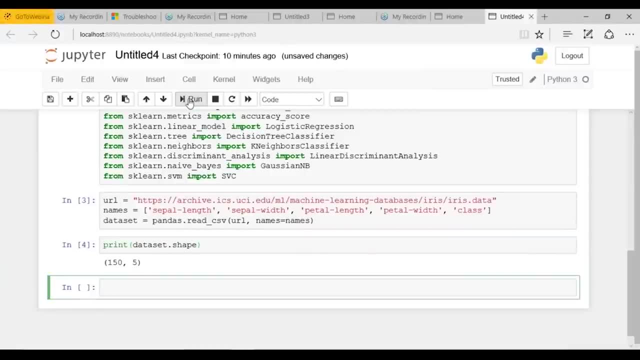 It will just give you the numbers of total number of rows and total number of column, or you can say the total number of instances or attributes in your data set. fine, So print data set dot shape, or do? you are getting 150 and 5. so 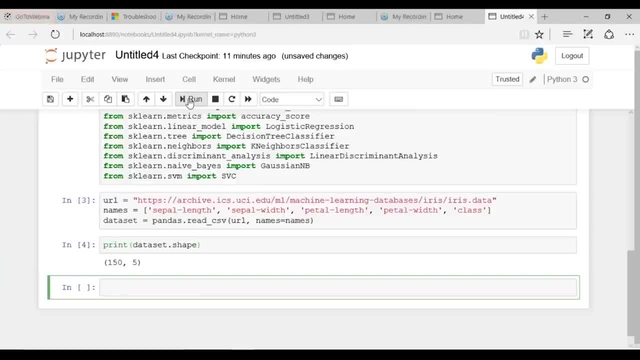 150 is the total number of rows in your data set and 5 is the total number of columns. fine, So moving on ahead, What if I want to see the sample data set? Okay, So let me just print the first 13 sizes of the data set. 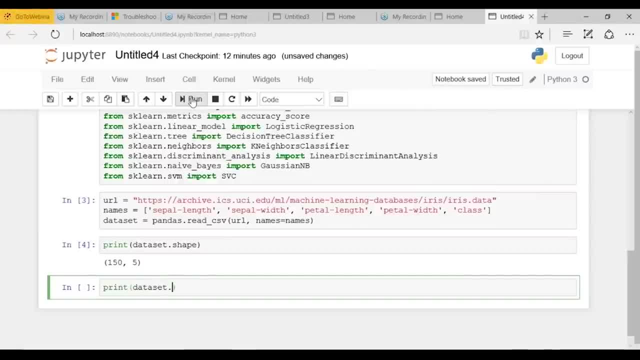 Okay, so print data set dot head. What I want is the first 30 instances. fine, This will give me the first 30 result of my data set. Okay, So when I hit the run button, what I am getting is the first 30. 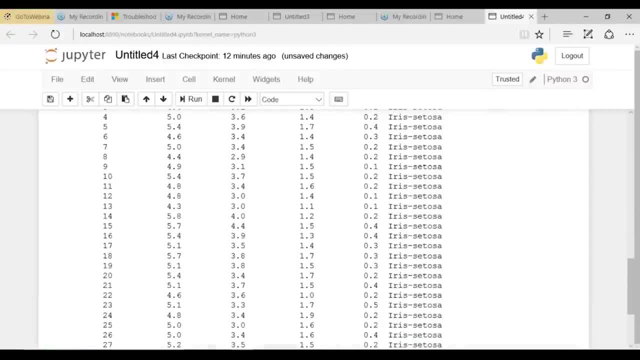 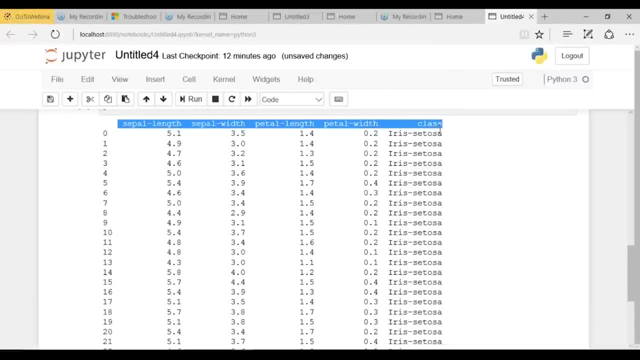 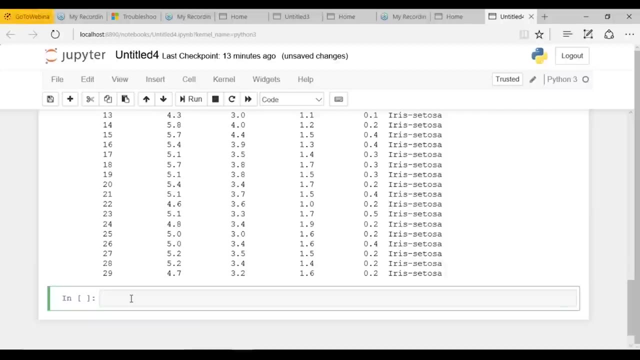 result: Okay, 0 to 29.. So this is how my sample data set looks like: separate, separate battle and battle with and the class: Okay, So this is how our data set looks like. now Let's move on and look at the summary of each attribute. 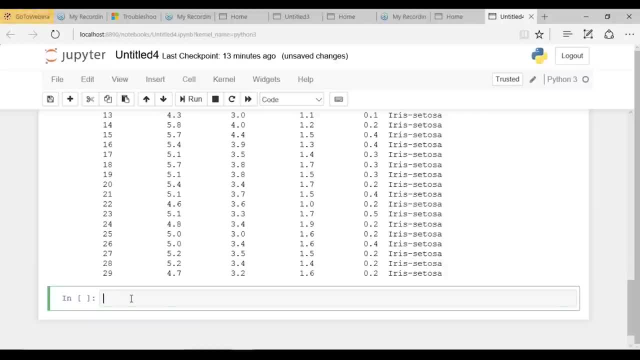 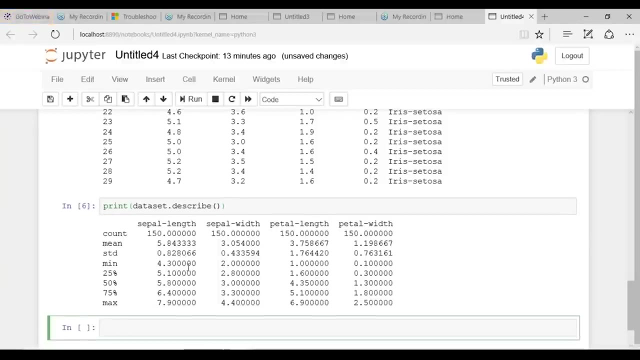 What if I want to find out? the count mean the minimum and the maximum values, and some other percentiles as well. So what should I do then for that print data set dot, describe What it will give. let's see. So you can see that all the numbers are the same scales of. 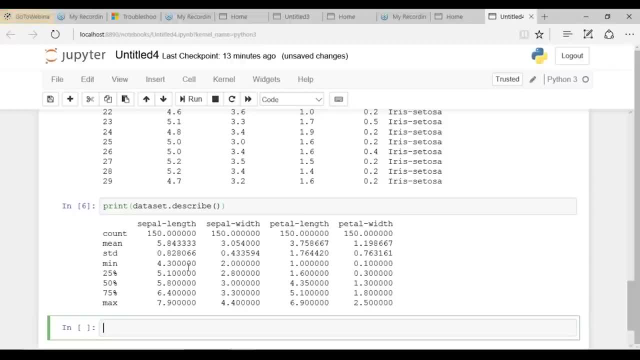 similar range between 0 to 8 centimeters. right. The mean value, the standard deviation, the minimum value, the 25 percentile, 50 percentile, 75 percentile, the maximum value. all these values lies in the range between 0 to 8 centimeter. 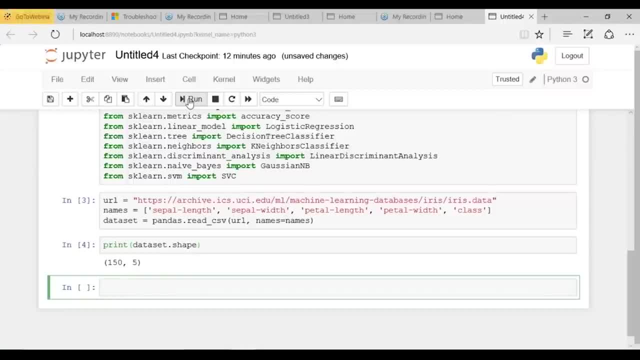 What if I want to see the sample Data set? Okay, So let me just print the first 13 sizes of the data set. Okay, so print data set dot head. What I want is the first 30 instances. fine, This will give me the first 30 result of my data set. 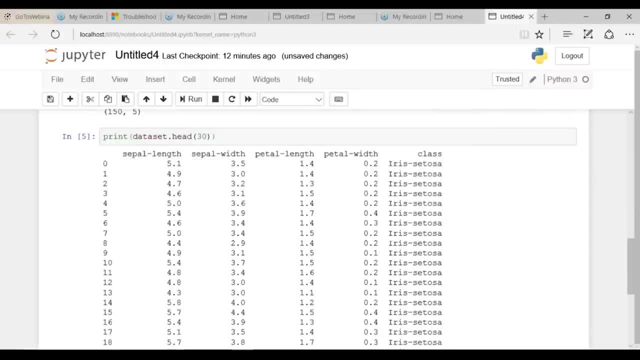 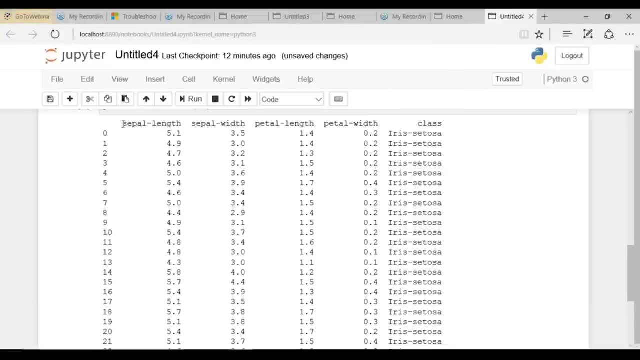 Okay. So when I hit the run button, what I am getting is the first 30 result: Okay, 0 to 29.. So this is how my sample data set looks like: sepal and separate petal and petal With, and the class. 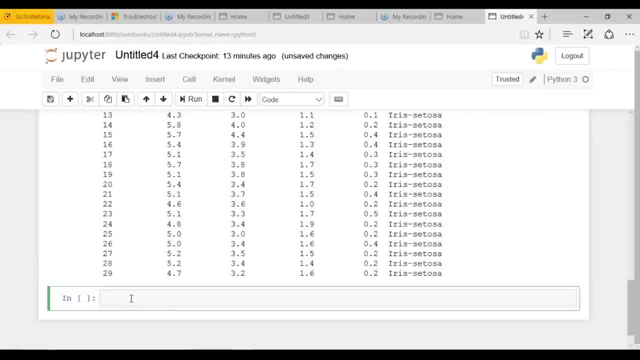 Okay, So this is how our data set looks like. now Let's move on and look at the summary of each attribute. What if I want to find out the count, mean, the minimum and the maximum values and some other percentiles as well? So what should I do then for that print data set? dot describe. 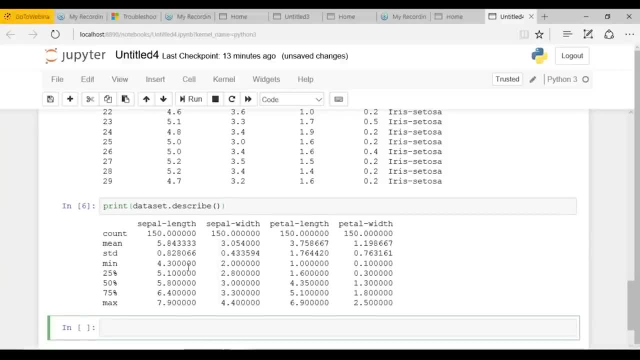 What it will give. let's see. So you can see that all the numbers are the same: scales of similar range between 0 to 8 centimeters. right, The mean value, the standard deviation, the minimum value, the 25 percentile, 50 percentile, 75 percentile, the maximum value. 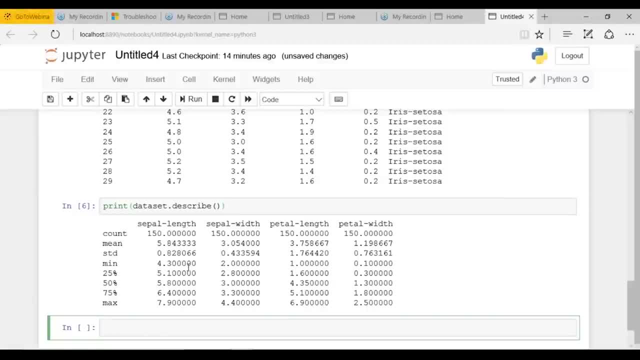 all these values lies in the range between 0 to 8 centimeter. Okay, So what we just did is we just took a summary of each attribute. now let's look at the number of instances that belong to each class. So for that, what we'll do: print data set first of all. 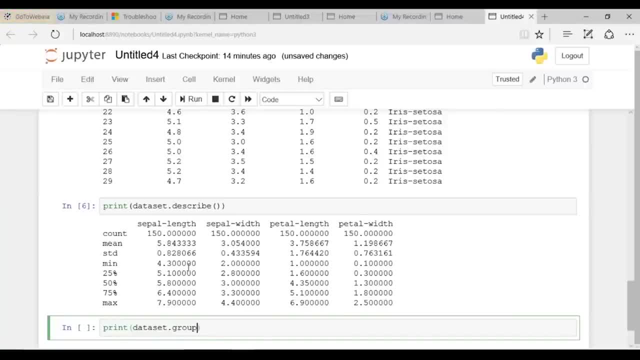 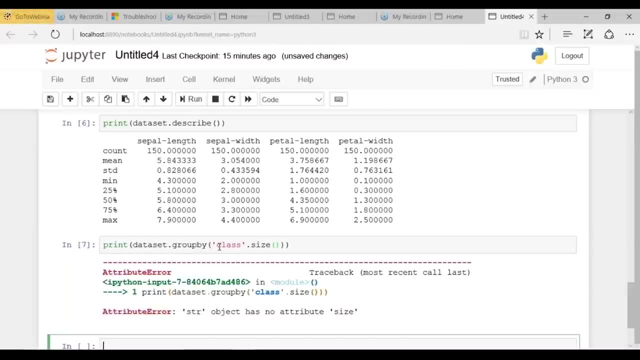 So let's print data set and I want to group it. So group by using class, and I want the size of it, size of each class, fine, and let's hit the run. Okay, So what I want to do? I want to print, print out data set, how I 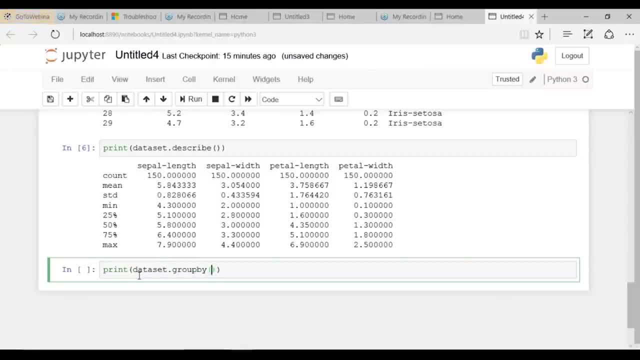 want to get it. I want it by class, So group by class. Okay, Now I want the size of each class. find the size of each class, So group by class, dot size and execute the run. So you can see that I have 15 stances of iris setosa, 15 stances. 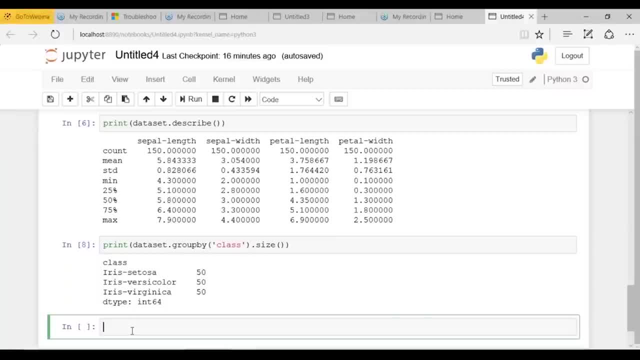 of iris versicolor and 15 stances of iris virginica. Okay, all are of data type integer of base 64. fine, So now we have a basic idea for data. Now let's move ahead and create some visualization for it. 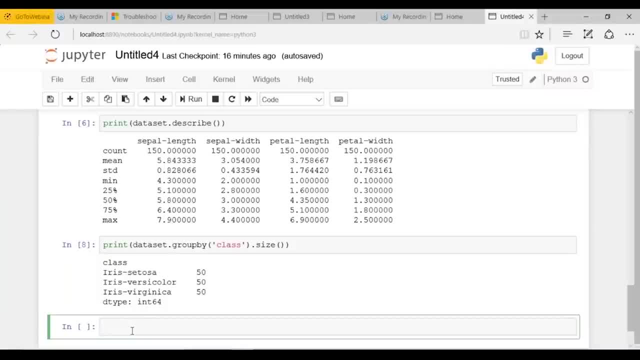 So for this we are going to create two different types of plot. first would be the univariate plot and the next would be the multivariate plot. So we'll be creating univariate plots to better understand about each attribute, and the next we'll be creating the. 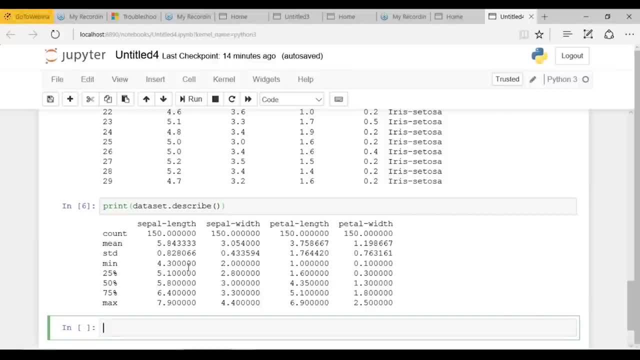 Okay, So what we just did is we just took a summary of each attribute. now let's look at the number of instances that belong to each class. So for that what we'll do: print data set first of all. So let's print data. 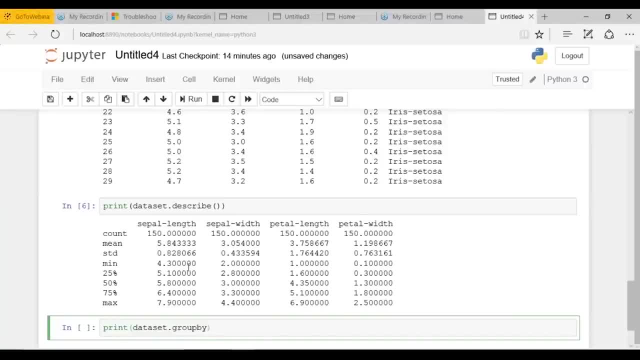 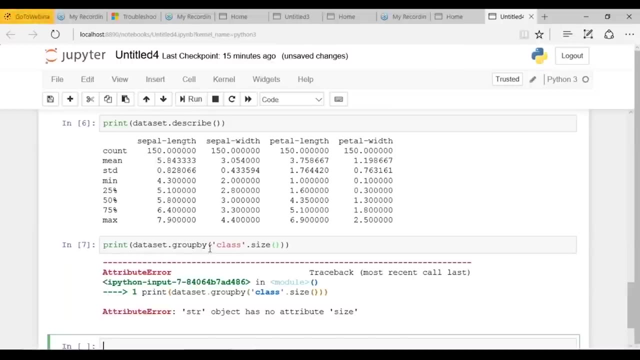 Set and I want to group it. group by using class, And I want the size of it, size of each class, fine, And let's hit the run. Okay, so what I want to do? I want to print. print what data set how I want to get it. 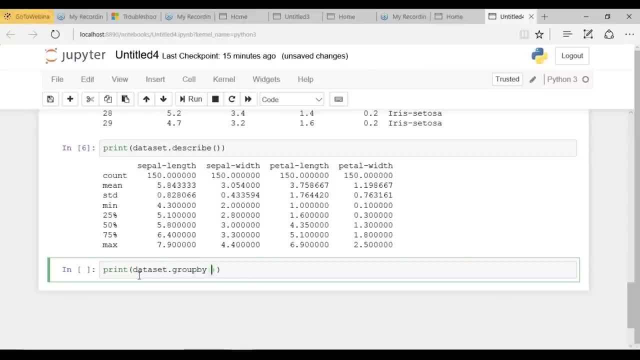 I want it by class, So group by class. Okay, Now I want the size of each class. find the size of each class, So group by class. dot size. execute the run So you can see that I have 15 stances of iris setosa: 15 stances. 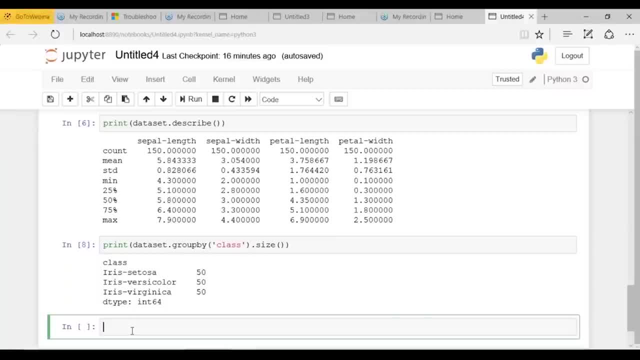 of iris versicolor and 15 stances of iris virginica. Okay, all are of data type integer of base 64. fine, So now we have a basic idea of our data. Now let's move ahead and create some visualization for it. 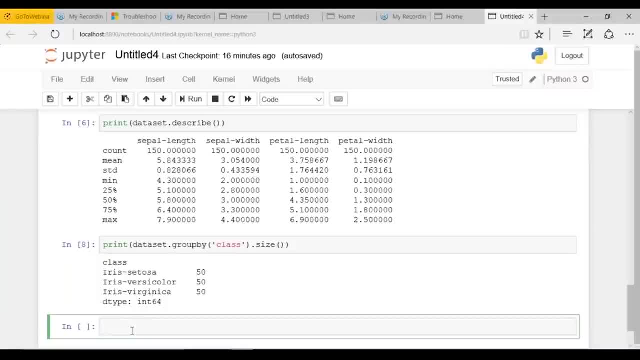 So for this we are going to create two Different types of plot. first would be the univariate plot and the next would be the multivariate plot. So we'll be creating univariate plots to better understand about each attribute, and the next will be creating the multivariate. 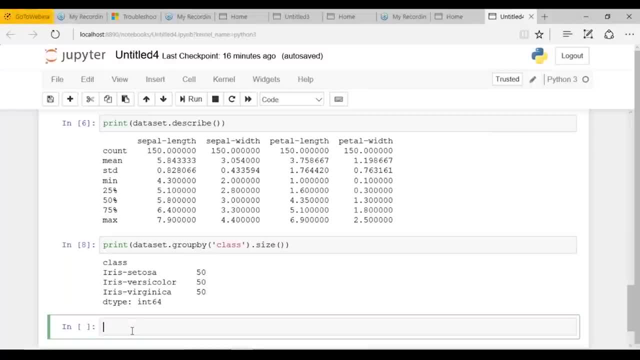 plot to better understand the relationship between different attributes. Okay so we start with some univariate plot, that is, plot of each individual variable. So, given that the input variables are numeric, we can create box and viscous plot for it. Okay so let's move ahead and create a box and viscous plot. 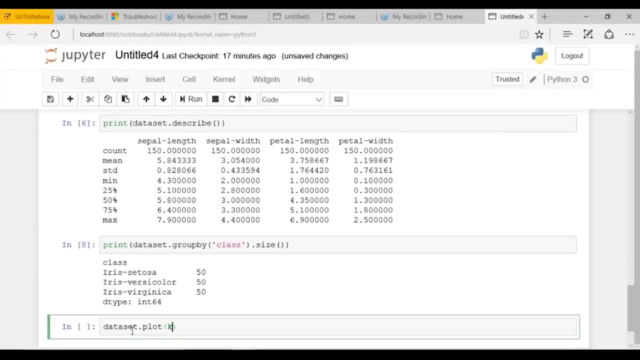 So data set, dot plot. What kind I want? it's a box, Okay. and do I need a subplot? Yeah, I need subplots for that. So subplots equal, true. What type of layout do I want? So my layout structure is 2 cross 2.. 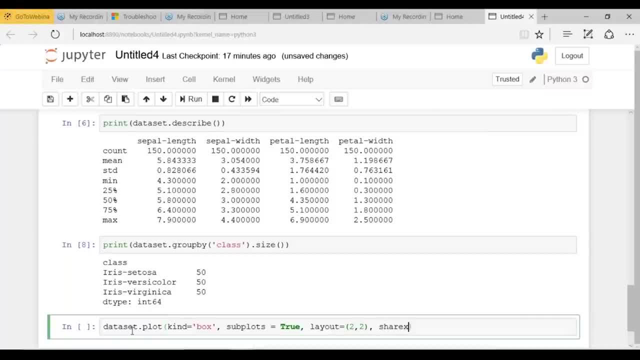 Next, do I want to share my coordinates, x and y coordinates? No, I don't want to share it. So share x equal false and even share y, that 2 equals false. Okay, so we have a data set dot plot kind equal box. 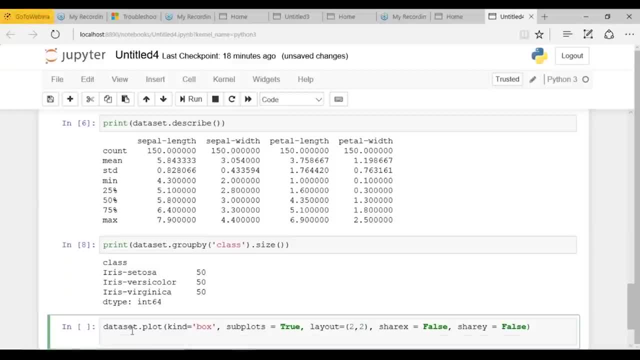 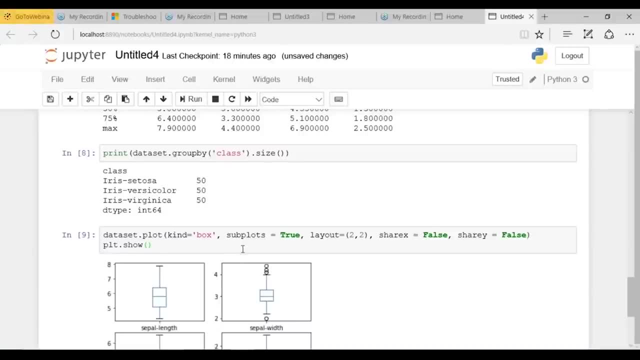 My subplots is true, layout 2 cross 2. and then what I want to do it. I want to see it. So, plot dot, show whatever I created. show it Okay, execute it Now. this gives us a much clearer idea about the distribution. 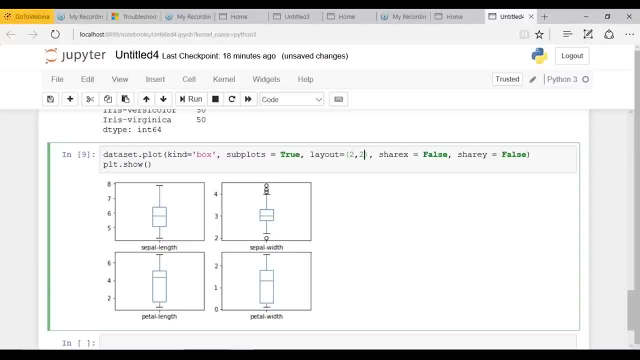 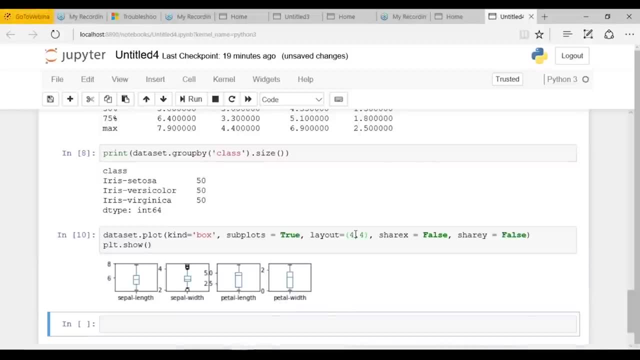 of the input attribute. Now what if I had given the layout to 2 cross 2? instead of that, I have given it 4 cross 4.. So what it will result? just see? fine, Everything would be printed in just one single row. 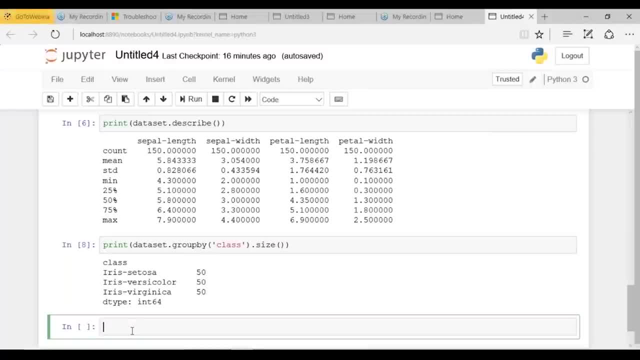 multivariate plot to better understand the relationship between different attributes. Okay so we start with some univariate plot, that is, plot of each individual variable. So, given that the input variables are numeric, we can create box and viscous plot for it. Okay so let's move ahead and create a box and viscous plot. 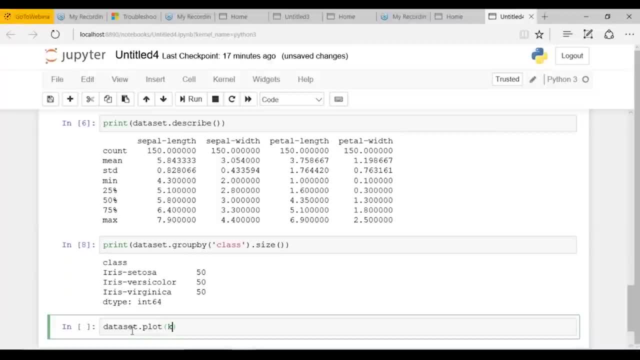 So data set, dot plot. what kind I want? it's a box, Okay. and do I need a subplot? Yeah, I need subplots for that. So subplots equals Well, true. What type of layout do I want? So my layout structure is 2 cross 2. next, 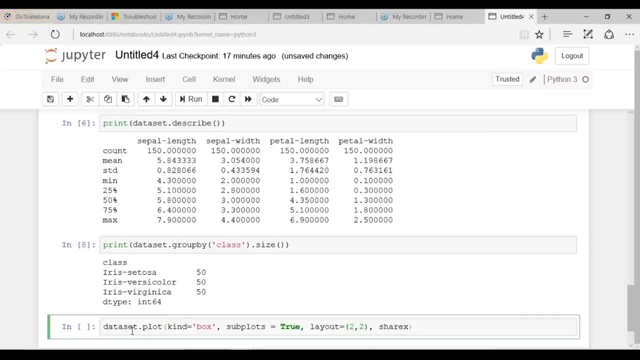 Do I want to share my coordinates, x and y coordinates? No, I don't want to share it. So share x equal false and even share y, that 2 equals false. Okay, so we have a data set dot plot kind equal box. 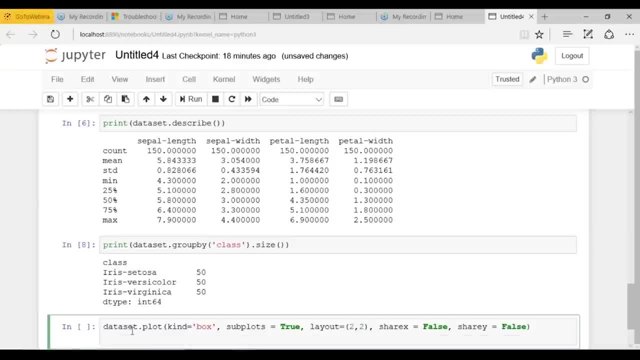 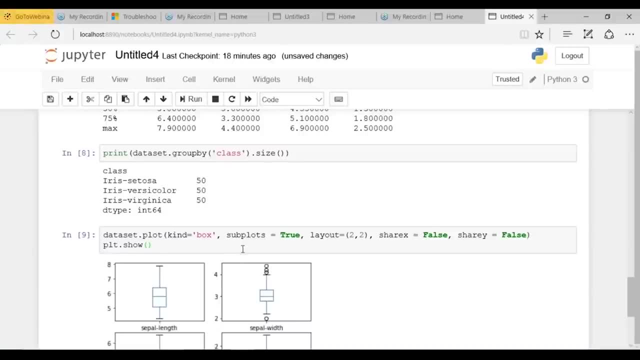 My subplots is true: layout 2 cross 2. and then what I want to do it? I want to see it. So, plot dot, show whatever I created. show it, Okay, Execute it Now. this gives us a much clearer idea about the distribution. 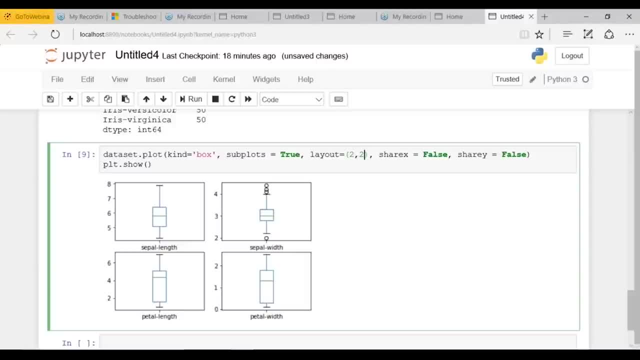 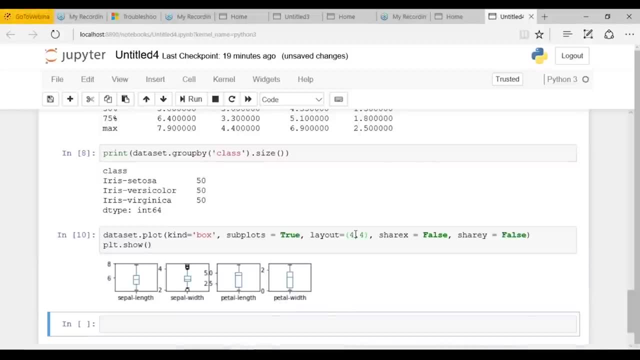 of the input attribute. Now what if I had given the layout to 2 cross 2? instead of that, I have given it 4 cross 4.. So what it will result? just see? fine, Everything would be printed in just one single row. 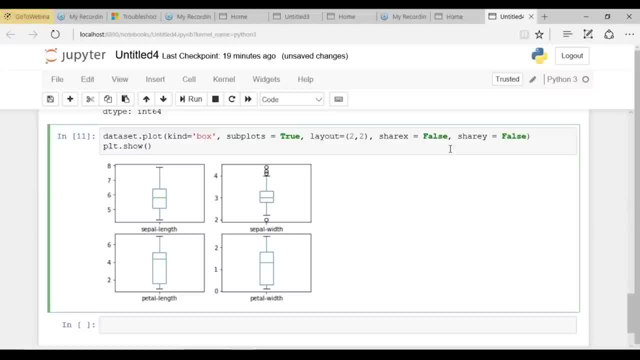 Hold on, guys. Aria is a doubt. He's asking that why we are using the share x and share y values. What are these? why we have assigned false values to it. Okay, area. So, in order to resolve this query, I need to show you what. 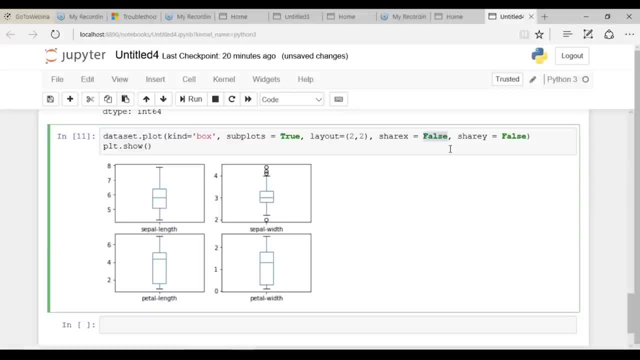 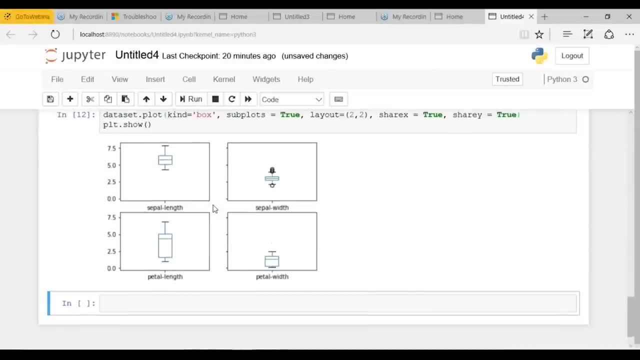 will happen if I give true values to them. Okay, so be with me. So share x- equal true, and share y, that equals true. So let's see what result will get. You're getting it. the x and y coordinates are just shared among all the four visualization right. 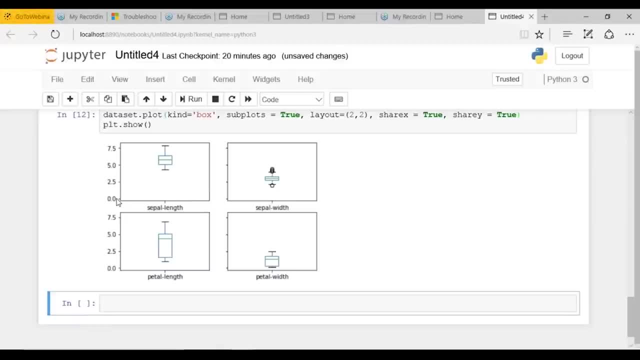 So already you can see that the sepal length and sepal width has y values ranging from 0.0 to 7.5, which are being shared among both. the visualization So is with the petal length: It has a shared value between 0.0 to 7.5.. 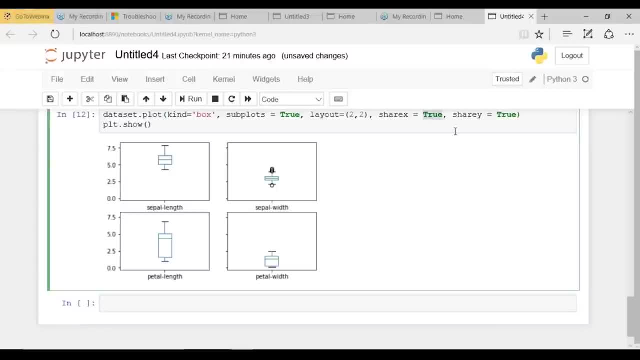 Okay, so that is why I don't want to share the value of x and y, So it's just giving us a cluttered visualization. So are you why I'm doing this? I'm just doing it because I don't want my x and y coordinates. 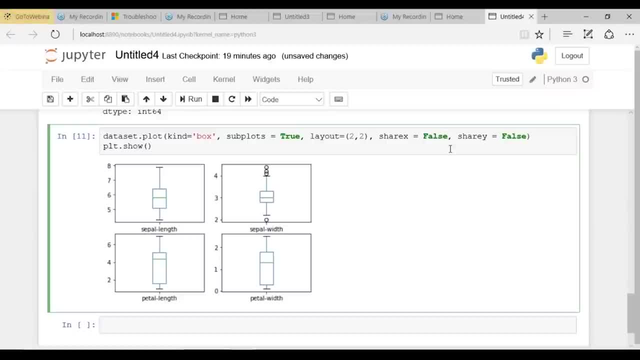 Hold on, guys. area is a doubt. He's asking that why we are using the share x and share y values. What are these? why we have assigned false values to it. Okay, area. So in order to resolve this query, I need to show you what will happen if I give true values. 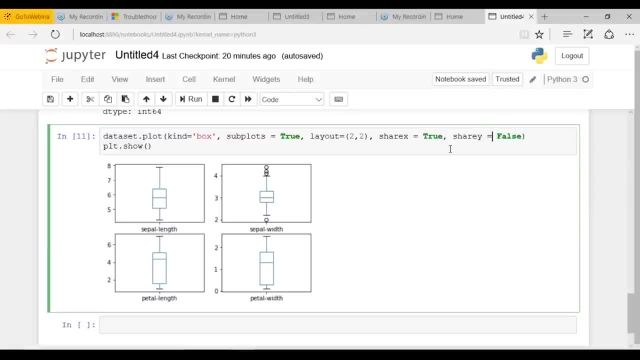 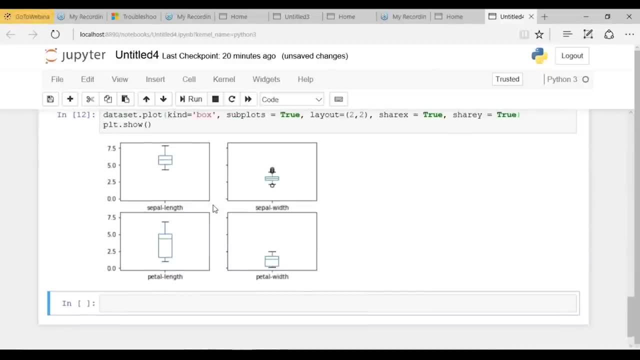 to them. Okay, so be with me. So share x- equal true, and share y- that equals true. So let's see what result will get. You're getting it. the x and y coordinates are just shared among all the four visualization right. 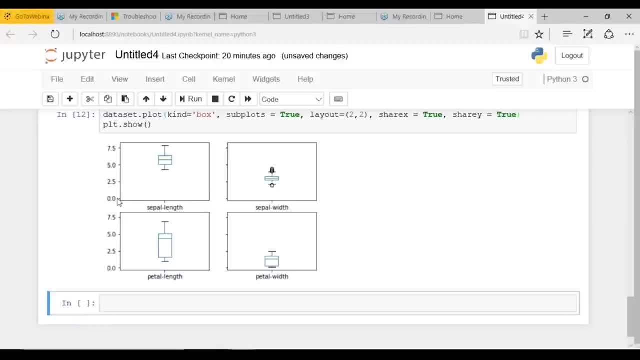 So already you can see that the sepal length and sepal width has y values ranging from 0.0 to 7.5, which are being shared among both. the visualization So is with the petal length: It has a shared value between 0.0 to 7.5.. 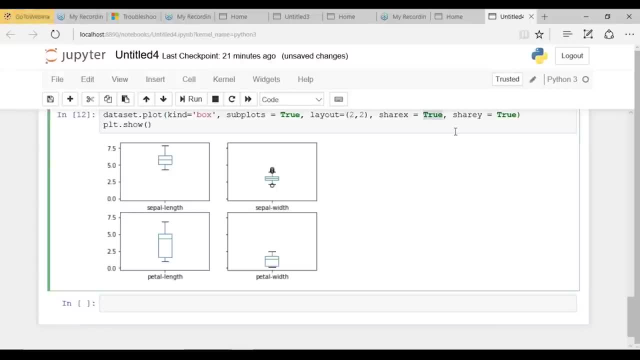 Okay, So that is why I don't want to share the value of x and y, so it's just giving us a cluttered visualization. So are you why I'm doing this? I'm just doing it because I don't want my x and y coordinates. 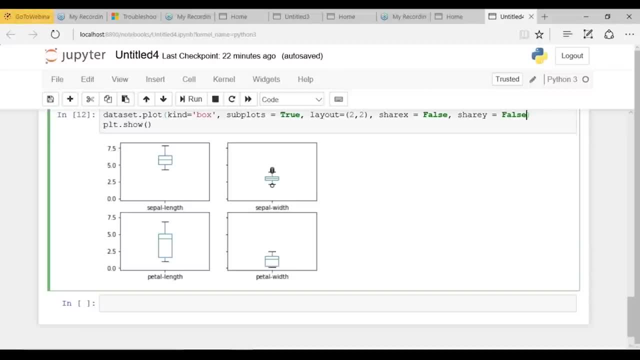 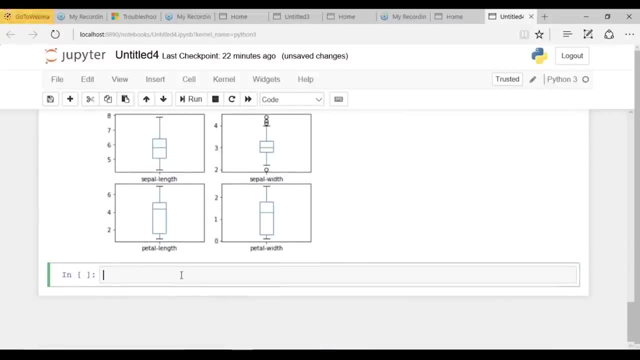 to be shared among any visualization. Okay, that is why my share x and share y value are false. Okay, let's execute it. So this is a pretty much clear visualization which gives a clear idea about the distribution of the input attributes. Now, if you want, you can also create a histogram of each input. 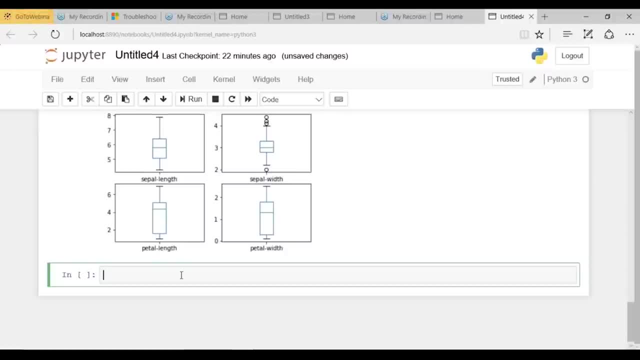 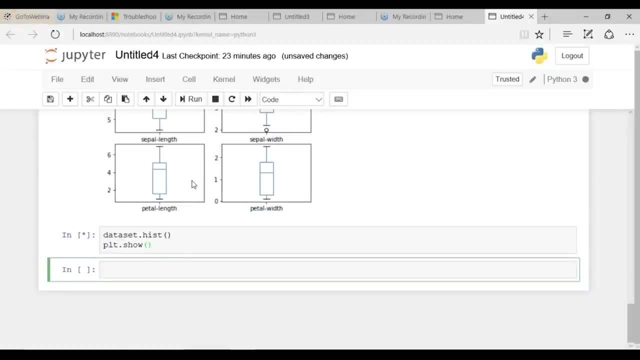 variable to get a clear idea of the distribution. So let's create a histogram for it. So data set dot hist. Okay, I would need to see it. So plot dot show- Let's see. So there's my histogram, and it seems that we have two input. 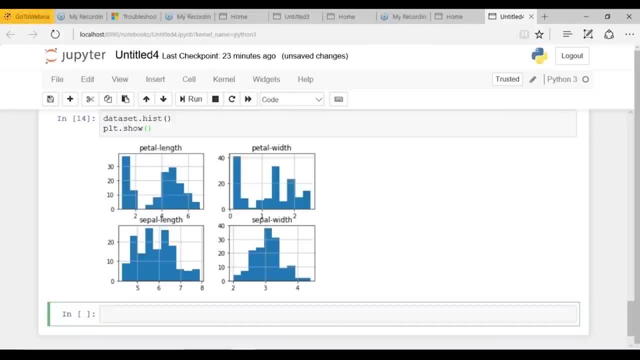 variables that have a Gaussian distribution. So this is useful to note as we can use the algorithms that can exploit this assumption. Okay, So next comes the multivariate plot. now that we have created the univariate plot to understand about each attribute, Let's move on and look at the multivariate plot and see the. 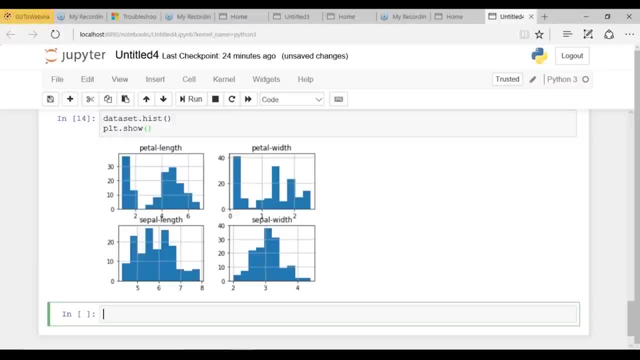 interaction between the different variables. So first let's look at the scatter plot of all the attributes. This can be helpful to spot structured relationship between input variables. Okay, so let's create a scatter matrix. So for creating a scatter plot we need scatter matrix and we 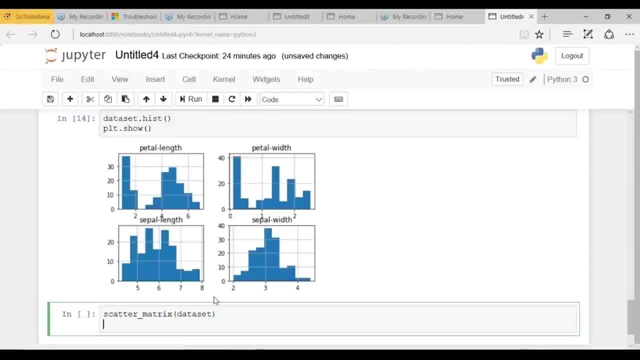 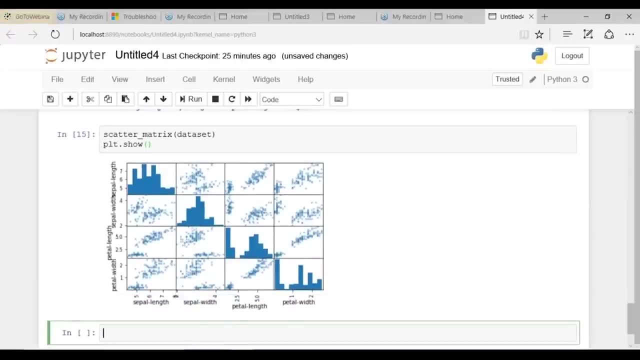 need to pass our data set into it. Okay, and then what I want? I want to see it so, plot dot show. So this is how my scatter matrix looks like. it's like that, the diagonal grouping of some pair, right. So this suggests a high correlation and a predictable relationship. 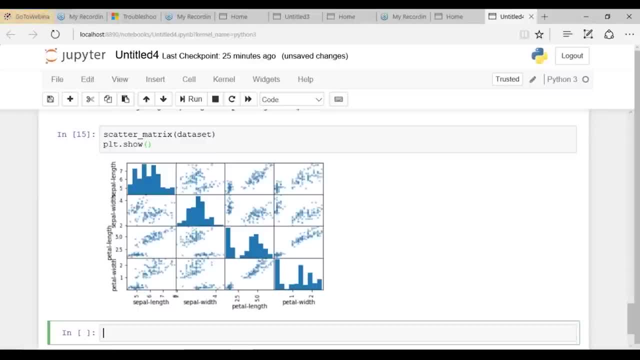 All right, This was our multivariate plot. Now let's move on and evaluate some algorithm. that's time to create some model of the data And estimate the accuracy on the basis of unseen data. Okay, So now we know all about our data set, right? 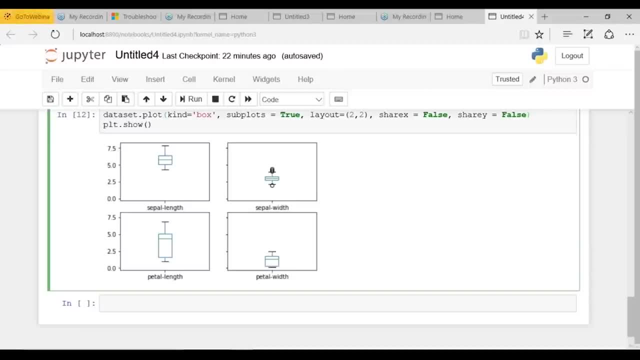 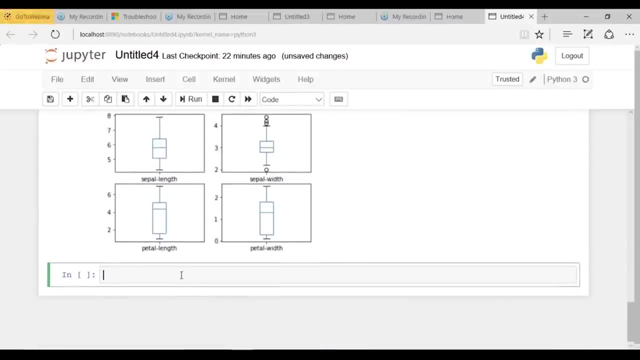 to be shared among any visualization. Okay, that is why my share x and share y value are false. Okay, let's execute it. So this is a pretty much clear visualization which gives a clear idea about the distribution of the input attributes. Now, if you want, you can also create a histogram of each input. 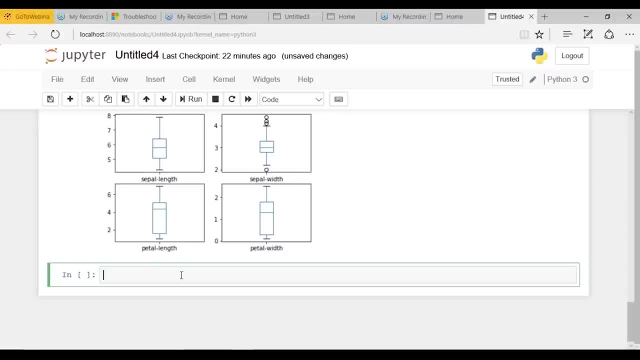 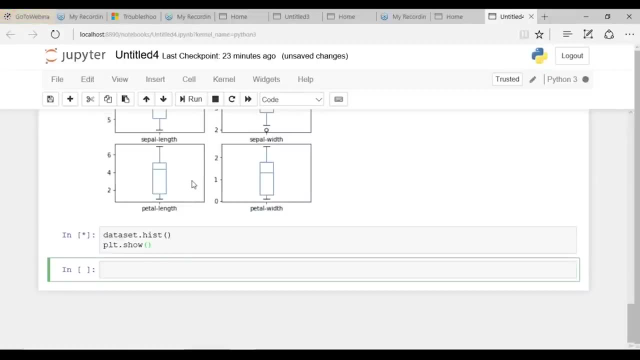 variable to get a clear idea of the distribution. So let's create a histogram for it. So data set dot hist. Okay, I would need to see it. So plot dot show- let's see. So there's my histogram, and it seems that we have two input. 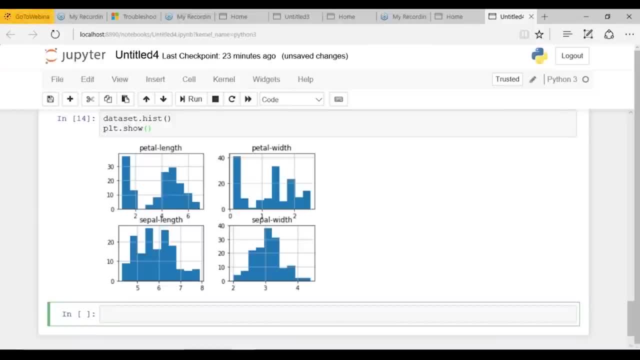 variables that have a Gaussian distribution. So this is useful to note as we can use the algorithms that can exploit this assumption. Okay, So next comes the multivariate plot. now that we have created the univariate plot to understand about each attribute, Let's move on and look at the multivariate plot and see the. 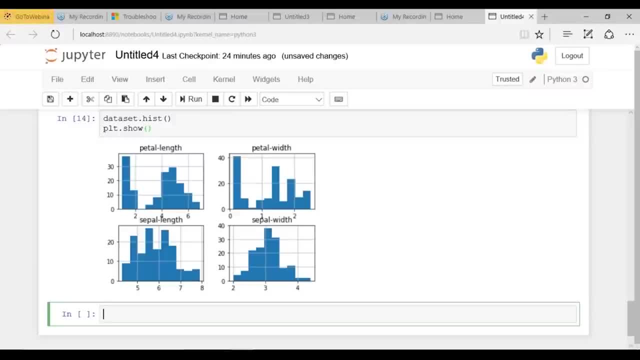 interaction between the different variables. So first let's look at the scatter plot of all the attribute. this can be helpful to spot structured relationship between input variables. Okay, So let's create a scatter matrix. So for creating a scatter plot we need scatter matrix and we 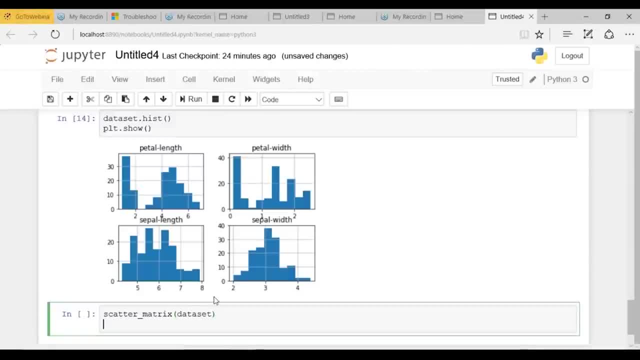 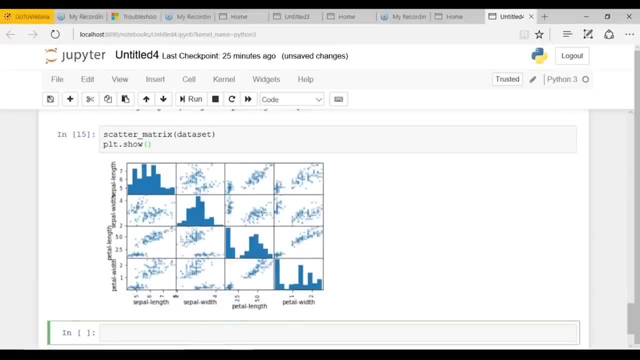 need to pass our data set into it. Okay, and then what I want? I want to see it so, plot dot show. So this is how my scatter matrix looks like. it's like that, the diagonal grouping of some pair, right. So this suggests a high correlation and a predictable. 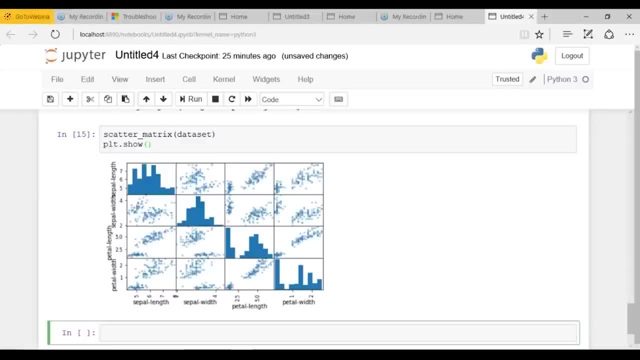 relationship. All right, this was our multivariate plot. Now let's move on and evaluate some algorithm. that's time to create some model of the data and estimate that accuracy on the basis of unseen data. Okay, So now we know all about our data set, right? 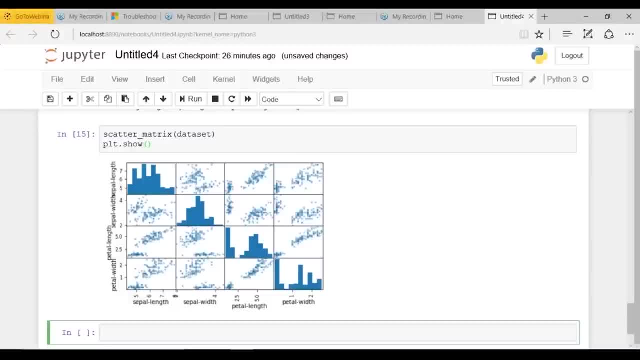 We know how many instances and attributes are there in our data set. We know the summary of each attribute. now I guess we have seen much about our data set. Now let's move on and create some algorithm and estimate their accuracy based on the unseen data. 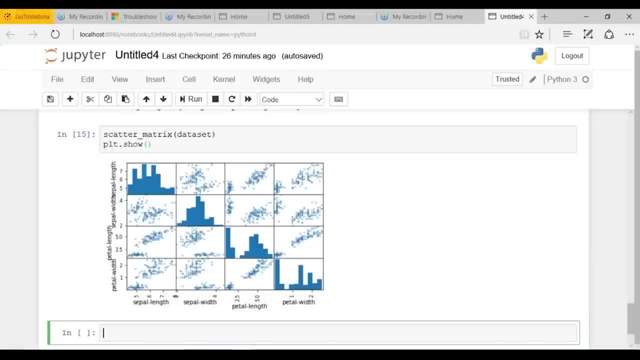 Okay, Now what we'll do will create some model of the data and estimate their accuracy based on the some unseen data. Okay, So for that, first of all, let's create a validation data set. What is the validation data set? validation data set is your. 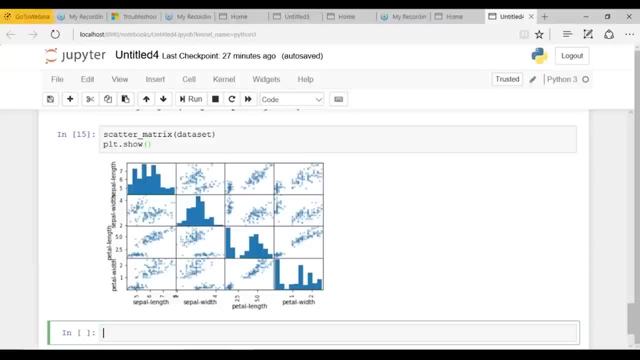 training data set that will be using it to train our model. Fine, All right. So how will create a validation data set? for creating a validation data set, What we are going to do is we are going to split our data set into two part. 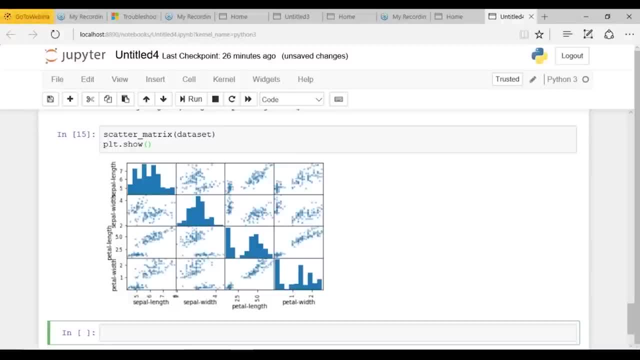 We know how many instances and attributes are there in our data set. We know the summary of each attribute. Now I guess we have seen much about our data set. Now let's move on and create some algorithm and estimate their accuracy based on the unseen data. 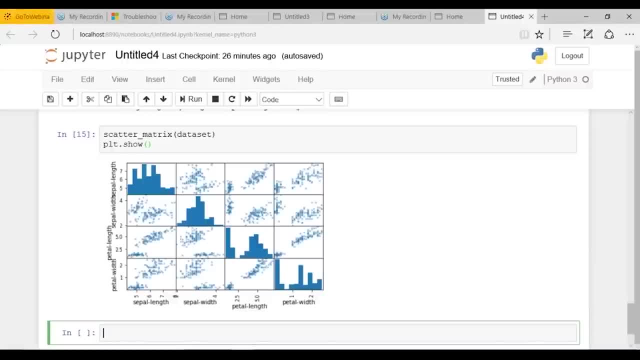 Okay, Now what we'll do will create some model of the data and estimate the accuracy based on the some unseen data. Okay, So for that, first of all, let's create a validation data set. What is a validation data set? validation data set. 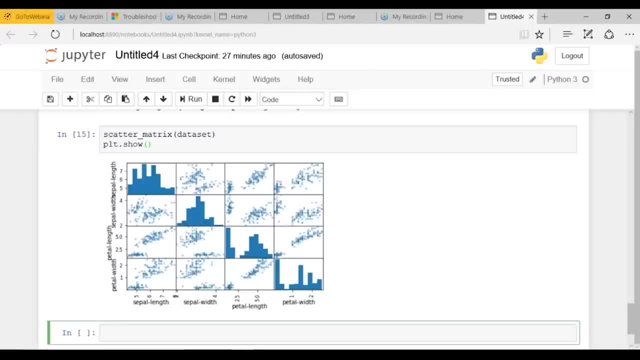 Is your training data set. that will be using it to train our model. Fine, All right. So how will create a validation data set? for creating a validation data set, What we are going to do is we are going to split our data set into two parts. 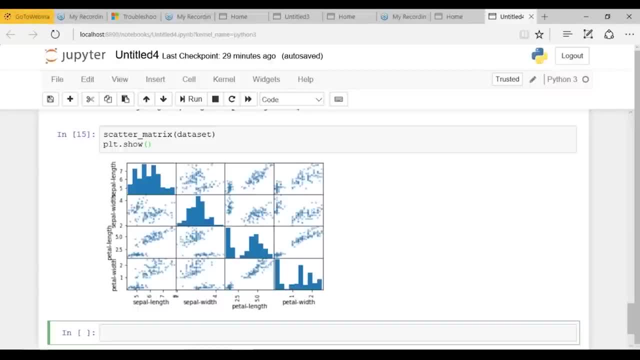 Okay, So the very first thing we'll do is to create a validation data set. So why do we even need a validation data set? So we need a validation data set. know that the model we created is any good. later, What we'll do will use the statistical method to estimate the 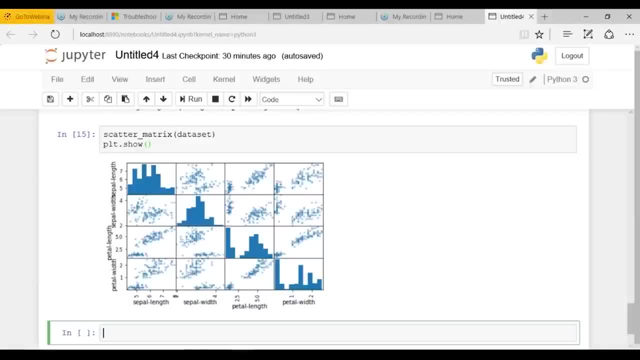 accuracy of the model that we create on the unseen data. We also want a more concrete estimate of the accuracy of the best model on unseen data by evaluating it on the actual unseen data. Okay, confused. Let me simplify this for you. What we'll do will split the loaded data into two parts. 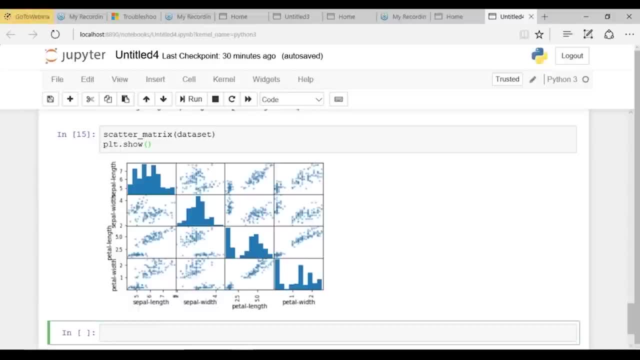 The first 80% of the data will use it to train our model and the rest 20% will hold back as the validation data set that will use it to verify our trained model. Okay, fine, So let's define an array. This is my array. what it will consist of? it will consist of: 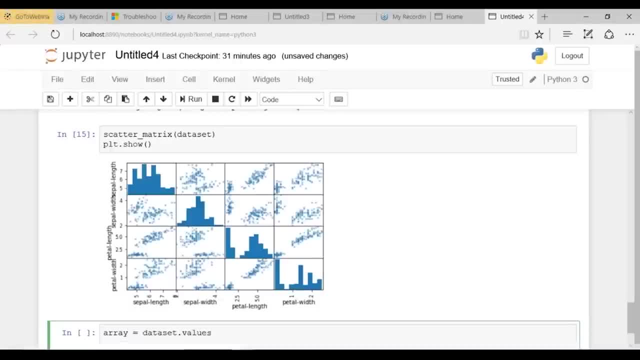 all the values from the data set. So data set, dot values. Okay, Next I'll define a variable X, which will consist of all the column from the array from 0 to 4, starting from 0 to 4, and the next variable Y, which would 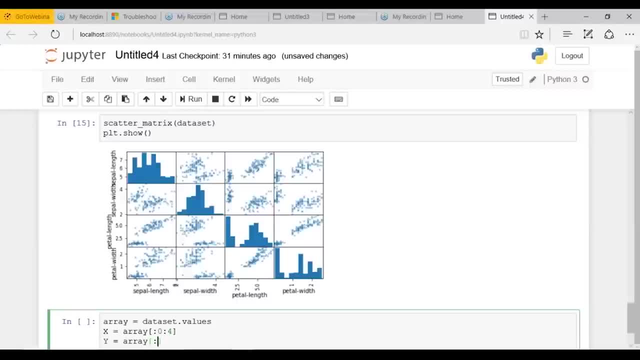 consist of the array starting from this. So, first of all, we'll define a variable X that will consist of the values in the array starting from the beginning, 0 till 4.. Okay, So these are the column which will include it in the X variable. 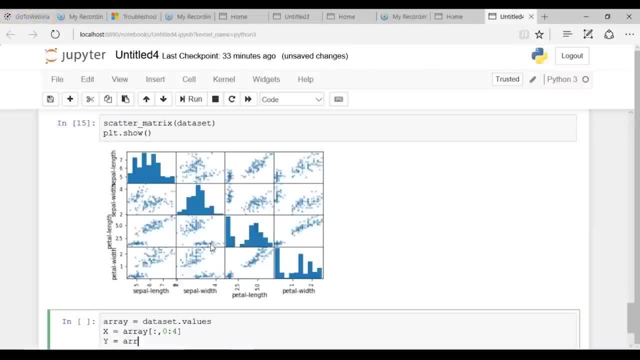 and for a Y variable, I'll define it as a class or the output. So what I need, I just need the fourth column. That is my class column. So I'll start it from the beginning and I just want the fourth column. 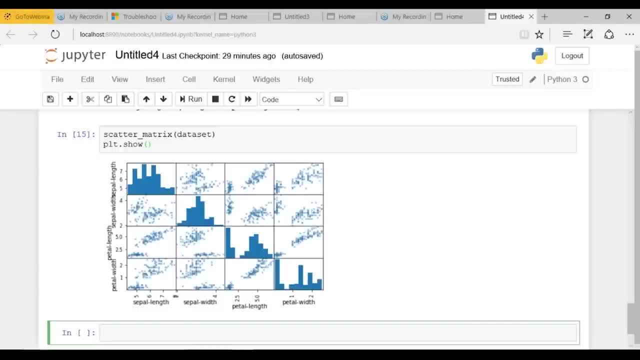 Okay, So the very first thing we'll do is to create a validation data set. So why do we even need a validation data set? So we need a validation data set. know that the model we created is any good. later, What we'll do will use the statistical method to estimate. 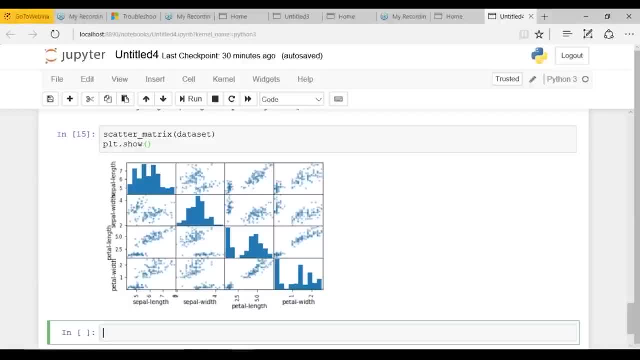 the accuracy of the model that we create on the unseen data. We also want a more concrete estimate of the accuracy of the best model on unseen data By evaluating it on the actual unseen data. Okay, confused. Let me simplify this for you. What we'll do will split the loaded data into two parts: the 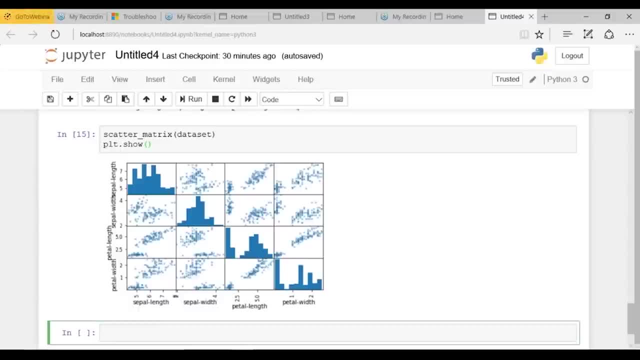 first, 80% of the data will use it to train our model and the rest 20% will hold back as the validation data set that will use it to verify our trained model. Okay, fine, So let's define an array. This is my array. what it will consist of? it will consist of: 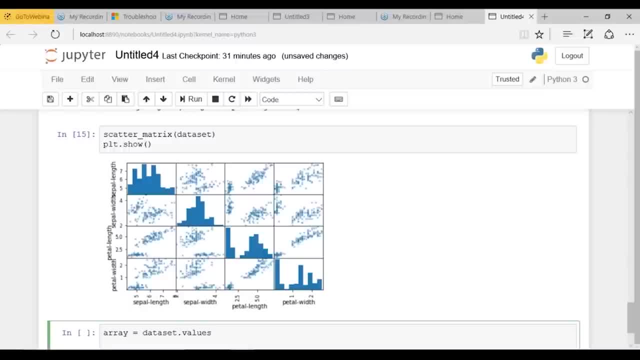 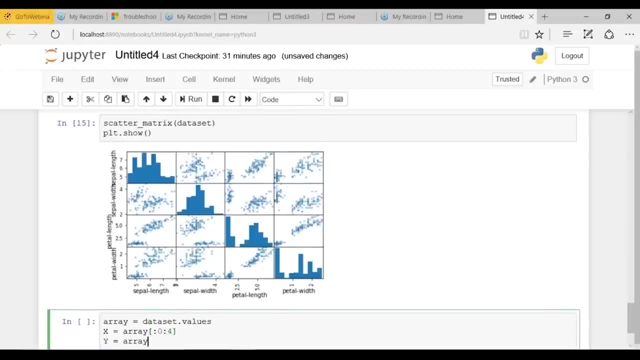 all the values from the data set. So data set, dot values. Okay, next I'll define a variable X, which will consist of all the column from the array, from 0 to 4, starting from 0 to 4, and the next variable Y, which would consist of the array. 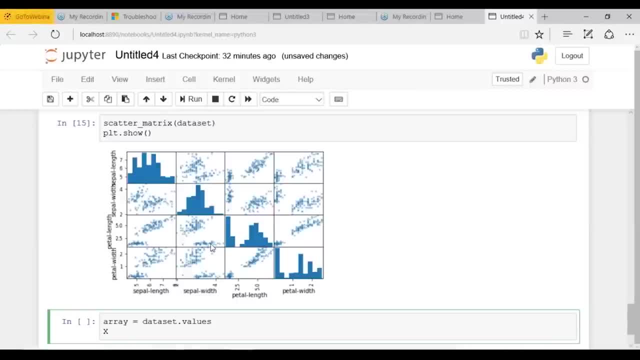 starting from this. So, first of all, we'll define a variable X that will consist of the values in the array starting from the beginning, 0 till 4.. Okay, So these are the column which will include it in the X variable and for a Y variable. 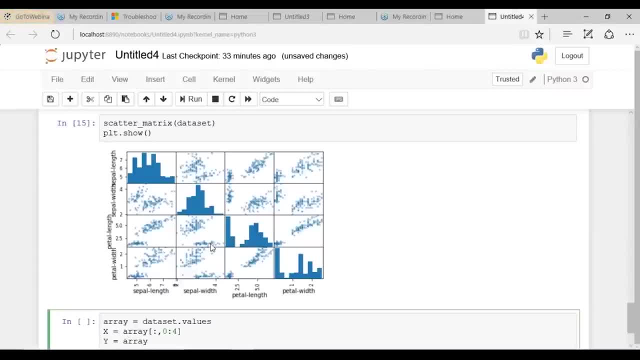 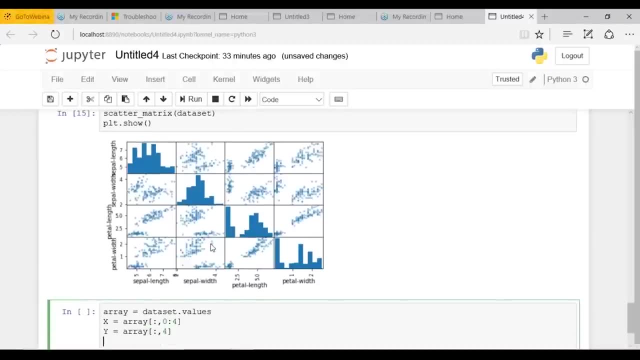 I'll define it as a class or the output. So what I need? I just need the fourth column. that is my class column. So I'll start it from the beginning and I just want the fourth column. Okay, now I'll define the, my validation, size, validation. 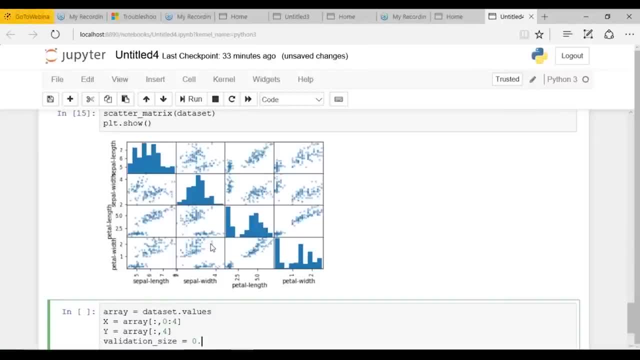 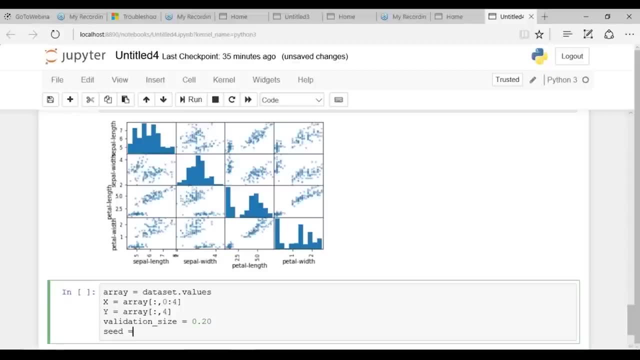 and a score size. I'll define it as 0.20 and I'll use a seed. I'll define seed equals 6.. So this method- seed- sets the integer starting value used in generating random number. Okay, I'll define the value of C equals 6.. 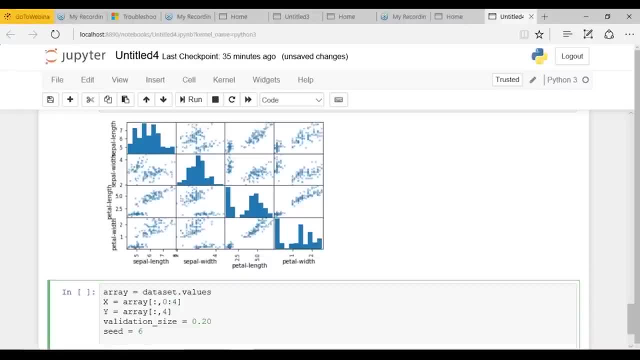 I'll tell you what is the importance of it later on. Okay, so let me define first few variables such as X and a score train test, Y underscore train and Y underscore test. Okay, So what do you want to do is select some model. 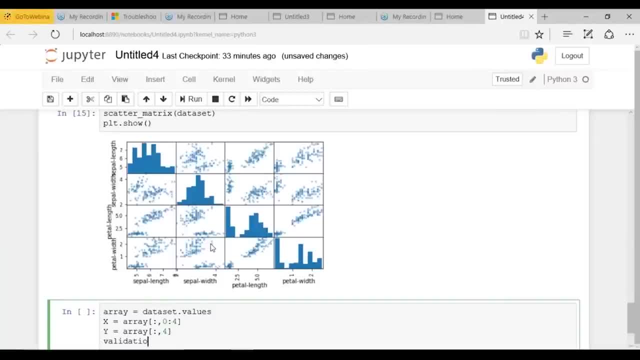 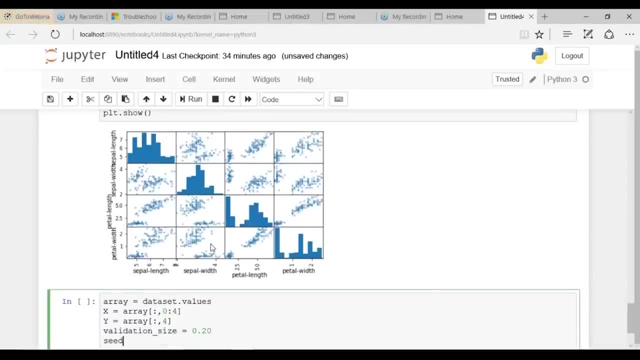 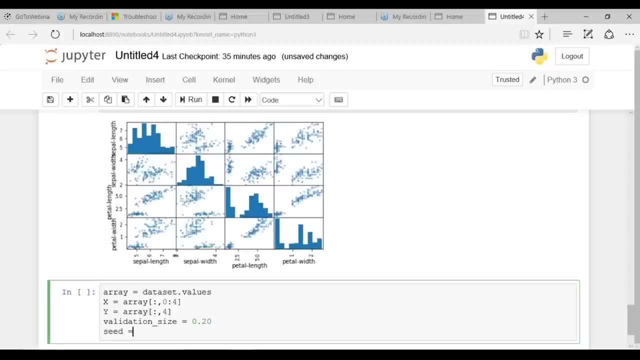 Okay, Now I'll Define my validation size- validation and a score size. I'll Define it as 0.20 and I'll use a seed. I'll Define seed equals 6.. So this method- seed- sets the integer starting value used in generating random number. 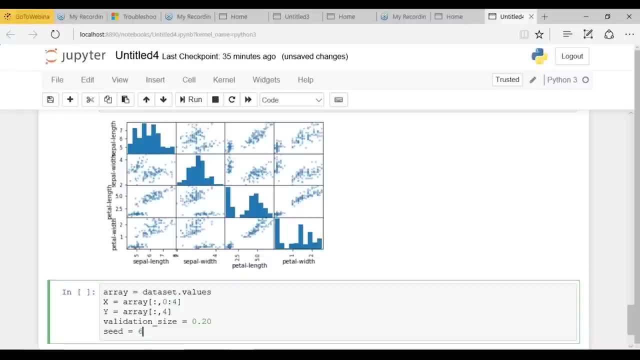 Okay, I'll Define the value of C equals 6.. I'll tell you what is the importance of it later on. Okay, So let me Define first few variables such as X underscore train test, Y underscore train and Y underscore test. Okay. 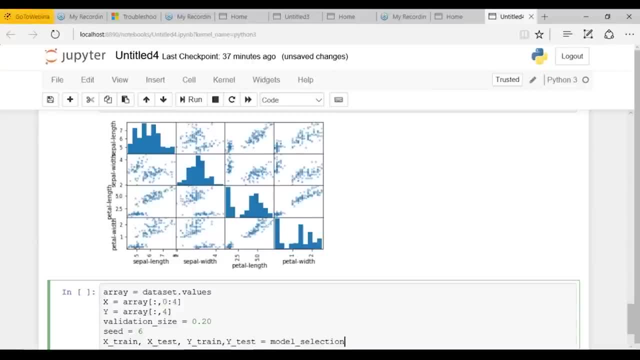 So what do we want to do is select some model. Okay so, model underscore selection. But before doing that, what we have to do is split our training data set into two hours. Okay so, dot train underscore, test underscore split. what we want to split is a value of X and Y. 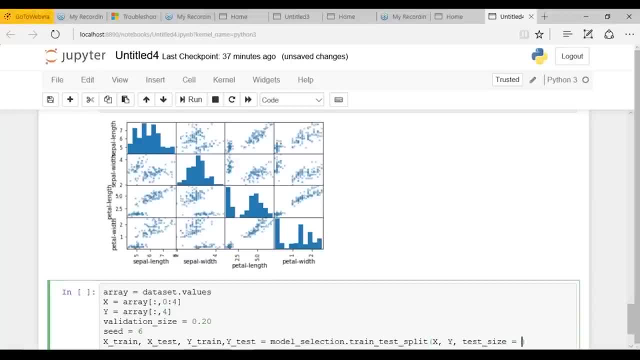 Okay, and my test size is equals to validation Size, which is a 0.20 correct, and my random state Is equal to seed. So what the seed is doing here? It's helping me to keep the same randomness in the training and testing data set. fine. 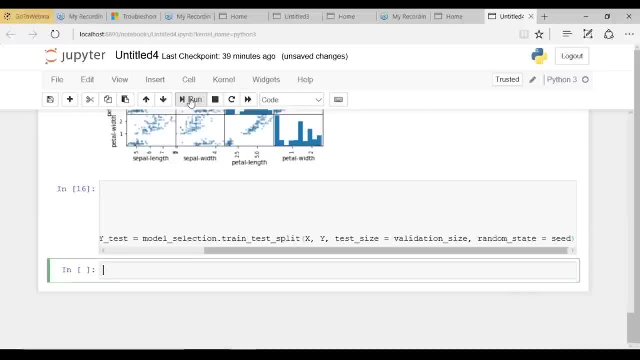 So let's execute it and see what is our result. It's executed. next will create a test harness for this, will use 10-fold cross validation to estimate the accuracy. So what it will do: it will split our data set into 10 parts, train on the nine part and test on the one part, and this will 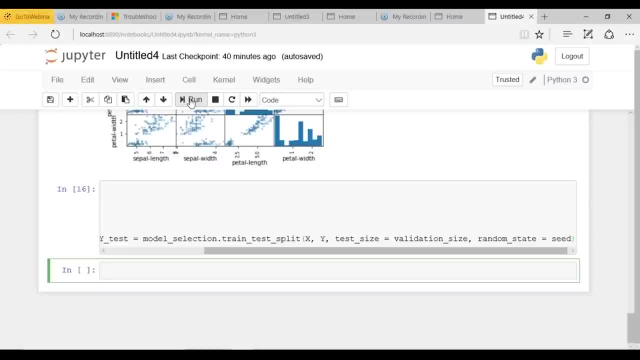 repeat, for all combination of train and test splits. Okay, So for that it's defined. again, my seed, that was six already defined, and scoring equals accuracy, fine, So we are using the metric of accuracy to evaluate the model. So what is this? There's a ratio of number of correctly predicted instances. 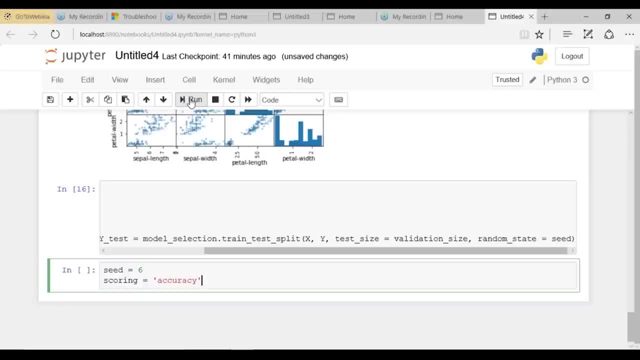 divided by the total number of instances in the data set, multiplied by hundred, Giving a percentage example, It's 98% accurate or 99% accurate, things like that. Okay, so we'll be using this scoring variable when we run the build and evaluate each model in the next step. 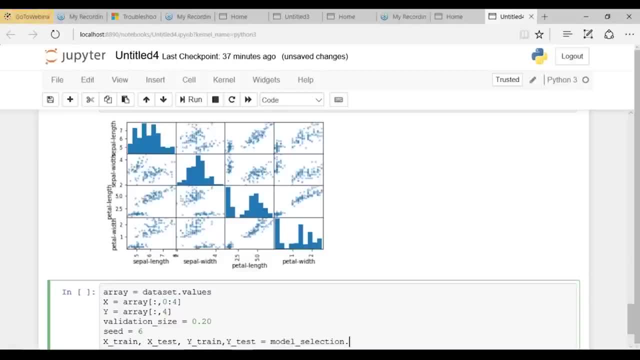 Okay, so model underscore selection. but before doing that, what we have to do is split our training data set into two hours. Okay, so dot train underscore, test underscore split. what we want to split is the value of X and Y. Okay, and my test size is equals to validation size, which is 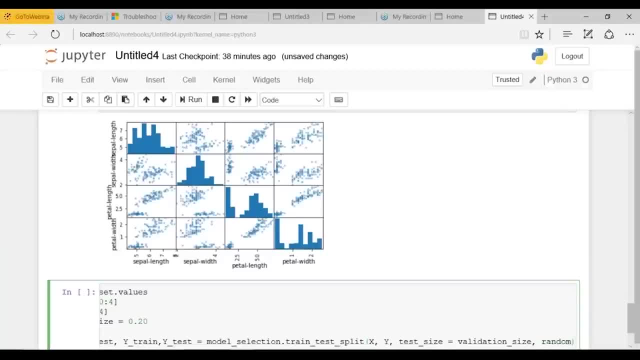 a 0.20.. So correct, and my random state Is equal to seed. So what the seed is doing here? It's helping me to keep the same randomness in the training and testing data set. fine, So let's execute it and see what is our result. 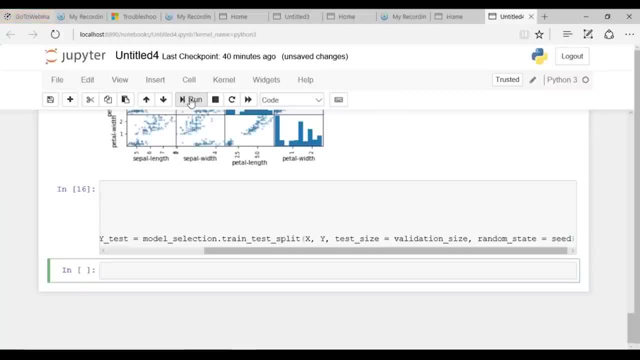 It's executed next will create a test harness for this, will use tenfold cross validation to estimate the accuracy. So what it will do? it will split our data set into ten parts, train on the nine part and test on the one part, and this will repeat for all combinations. 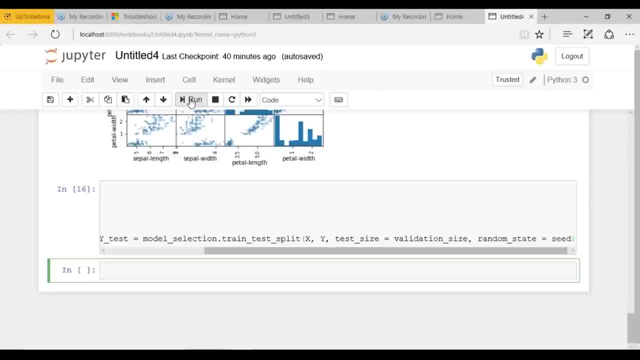 Of train and test splits. Okay, So for that it's defined. again, my seed, that was six already defined, and scoring equals accuracy, fine, So we are using the metric of accuracy to evaluate the model. So what is this? There's a ratio of number of correctly predicted instances. 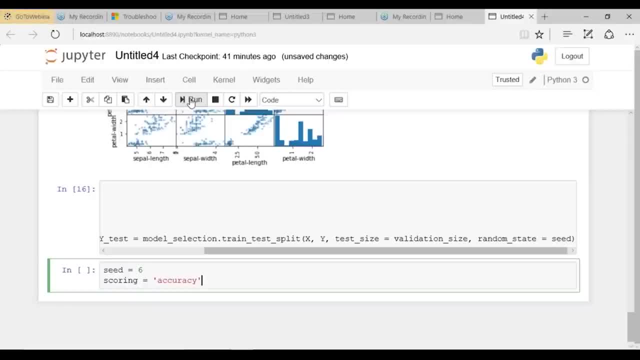 divided by the total number of instances in the data set, multiplied by hundred, giving a percentage example, it's 98% accurate or 99% Accurate, things like that. Okay, so we'll be using this scoring variable when we run the build and evaluate each model in the next step. 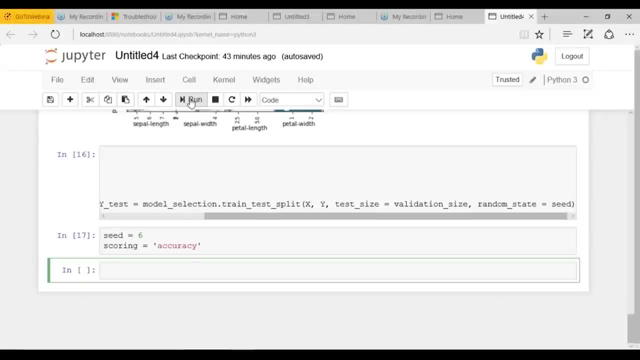 So next part is building model. till now, We don't know which algorithm would be good for this problem or what configuration to use, So let's begin with six different algorithm. I'll be using logistic regression, linear discriminant analysis- k nearest neighbor classification and regression trees- neighbors. 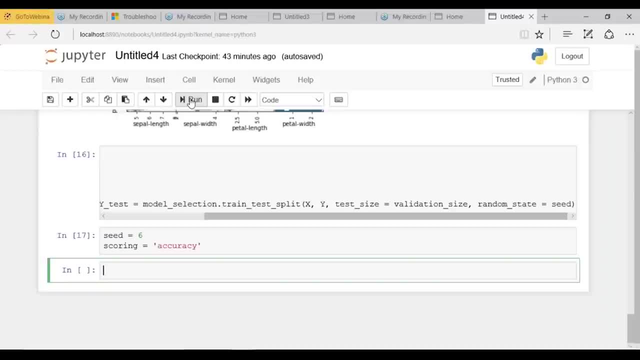 and code vector machine. Well, these algorithms chime using is a good mixture of simple linear or nonlinear algorithms. and simple linears, which included the logistic regression and the linear discriminant analysis, or the nonlinear part, which included the KNN algorithm, the cart algorithm that the neighbors and the support vector. 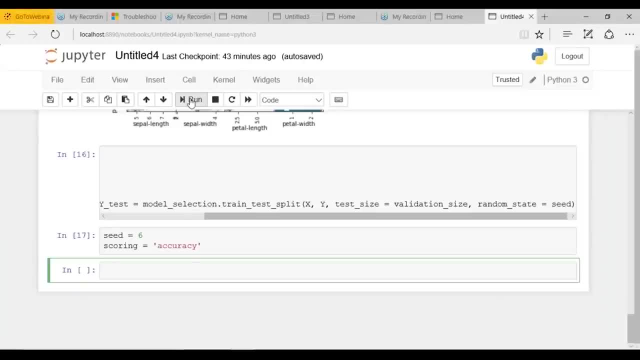 So next part is building model. till now, We don't know which algorithm would be good for this problem or what configuration to use, So let's begin with six different algorithm. I'll be using logistic regression, linear discriminant analysis, k nearest neighbor classification and regression trees- nabias. 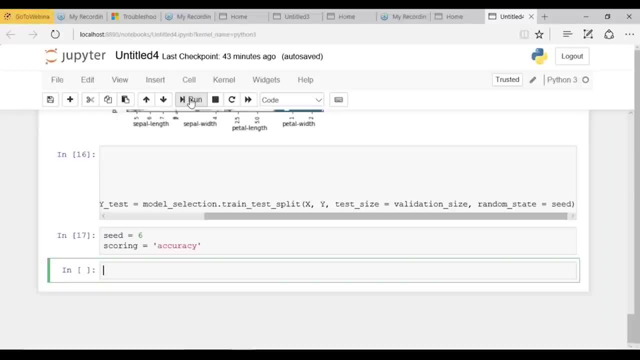 and code vector. Well, these algorithms chime using is a good mixture of simple linear or nonlinear algorithms. and simple linears, which included the logistic regression and the linear discriminant analysis, or the nonlinear part, which included the KNN algorithm, the cart algorithm that the neighbor is. 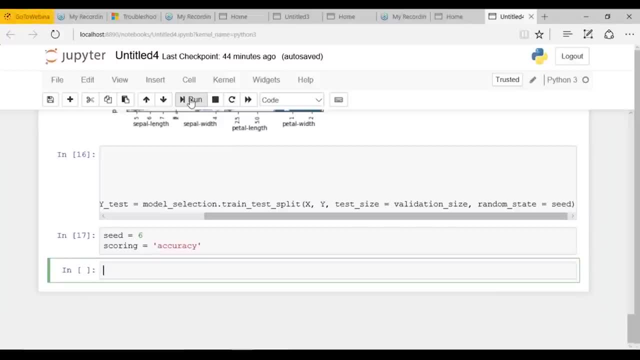 and the support vector machines. Okay, so we reset the random number seed before each run to ensure that evaluation of each algorithm is performed using exactly the same data splits. It ensures the result are directly comparable. Okay, so let me just copy and paste it. 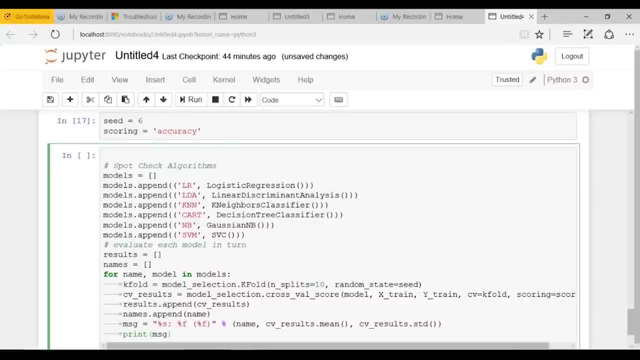 Okay, So what we are doing here? we are building five different types of model. We are building logistic regression, linear discriminant analysis, k nearest neighbor, legend tree, Gaussian, a bias and the support vector machine. Okay, Next, what we'll do will evaluate model in each turn. 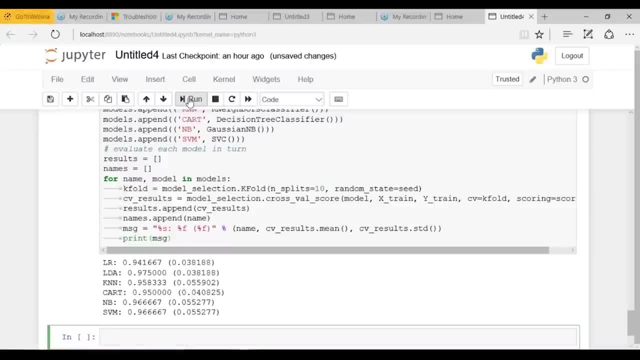 Okay, So what is this? So we have six different model and accuracy estimation for each one of them. Now we need to compare the model to each other and select the most accurate of them all. So, running this script, We saw the following result: 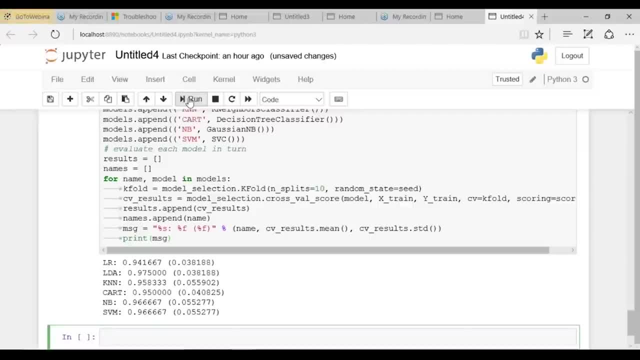 So we can see some of the result on the screen. What is this? It is just the accuracy scored using different set of algorithms. Okay, when we are using logistic regression, what is the accuracy rate when we are using near discriminant algorithm? 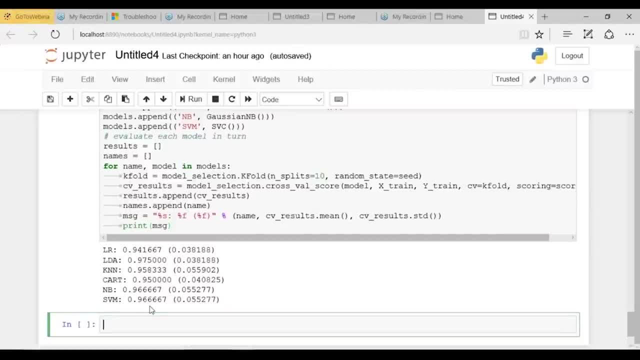 What is the accuracy, and so on. So okay, so from the output it seems that LDL got them was the most accurate model that we tested. now We want to get an idea of the accuracy of the model on our validation set or the testing data set. 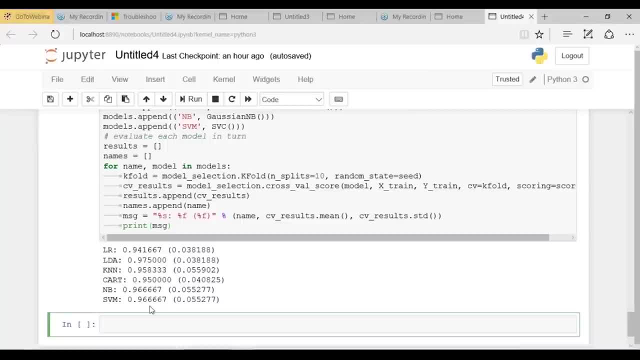 So this will give us a independent final check on the accuracy of the best model. It is always valuable to keep our testing data set for just in case you made a overfitting to the testing data set or you made a data leak. both will result in a overly optimistic. 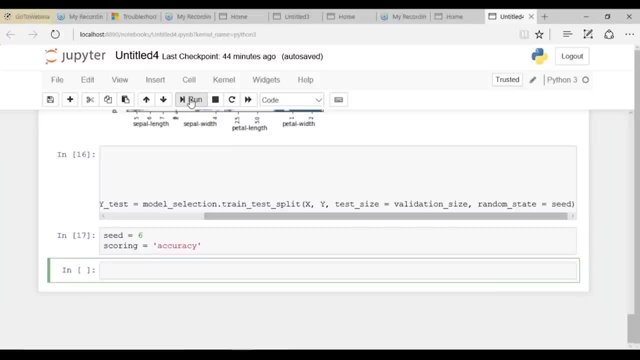 machines. Okay, so we reset the random number seed before each run to ensure that evaluation of each algorithm is performed using exactly the same data spreads. It ensures the result are directly comparable. Okay, so let me just copy and paste it: Okay. 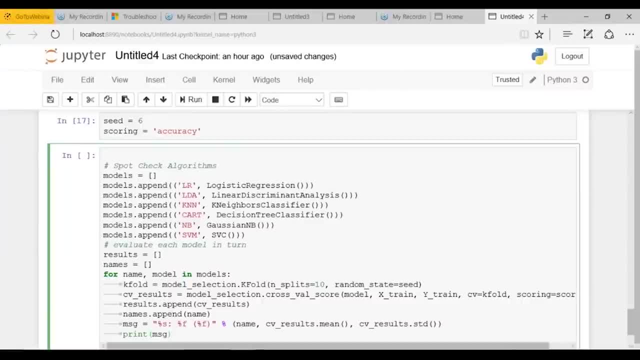 So what we are doing here, We are building five different types of model. We are building logistic regression, linear discriminant analysis, k nearest neighbor, decision tree, Gaussian, a bias and the support vector machine. Okay, Next, what we'll do will evaluate model in each turn. 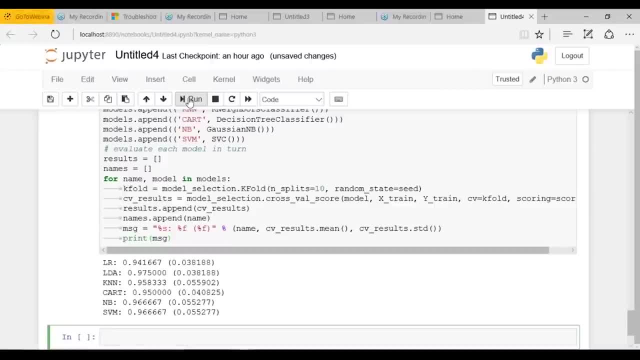 Okay, So what is this? So we have six different model and accuracy estimation for each one of them. Now we need to compare the model to each other and select the most accurate of them all. so, running this script, We saw the following result. so we can see some of the result. 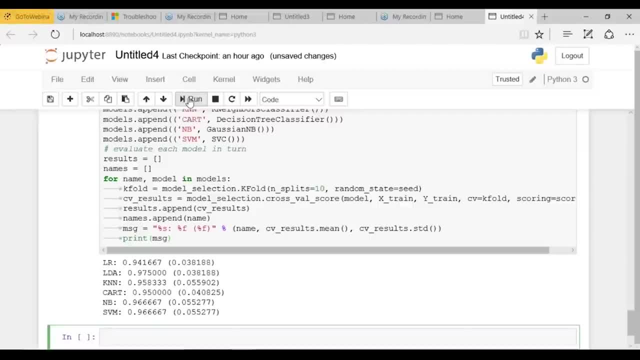 on the screen. What is this? It is just the accuracy score using different set of algorithms. Okay, when we are using logistic regression, what is the accuracy rate? when we are using near discriminant algorithm, What is the accuracy? and so on. so okay, 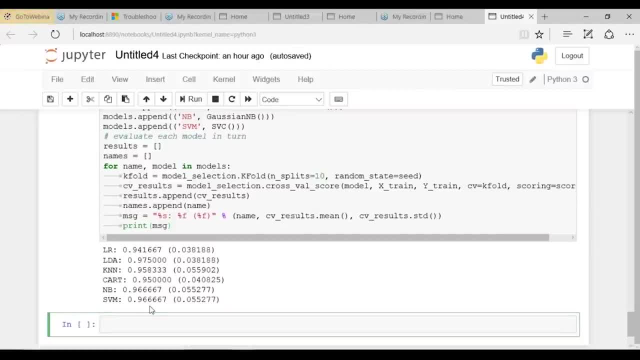 So from the output it seems that LDL got them was the most accurate model that we tested. now We want to get an idea of the accuracy of the model on our validation set or the testing data set. So this will give us a independent final check on the. 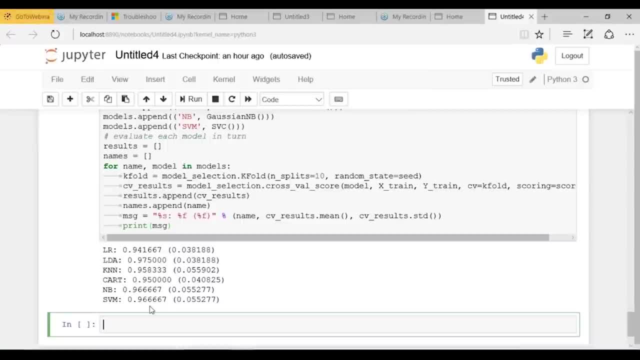 accuracy of the best model. It is always valuable to keep our testing data set for just in case you made a overfitting to the testing data set or you made a data leak. both will result in a overly optimistic result. Okay, you can run the LDL model directly on the validation set. 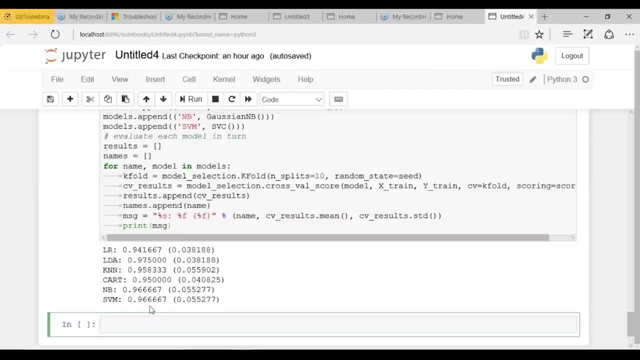 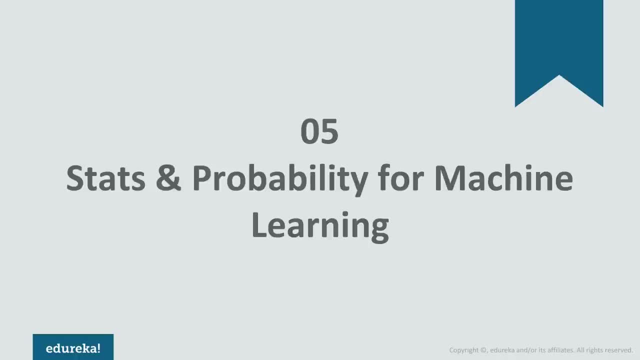 and summarize the result as a final score, a confusion Matrix and a classification report. Statistics and probability are essential because these disciples form the basic foundation of all machine learning, algorithms, deep learning, artificial intelligence and data science. In fact, mathematics and probability is behind everything around us, from shapes, patterns and colors to the count of. 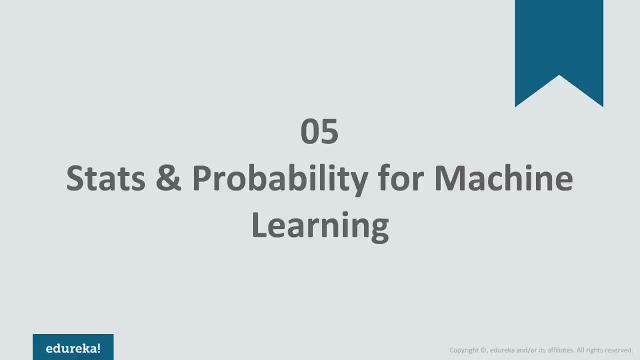 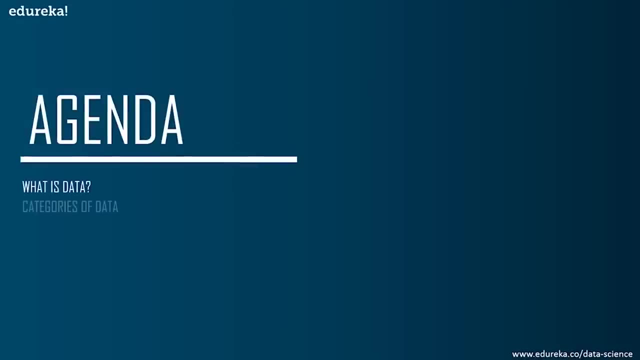 petals in a flower. mathematics is embedded in each and every aspect of our lives, So I'm going to go ahead and discuss the agenda for today with you all. We're going to begin the session by understanding What is data. after that, We'll move on and look at the different categories of data. 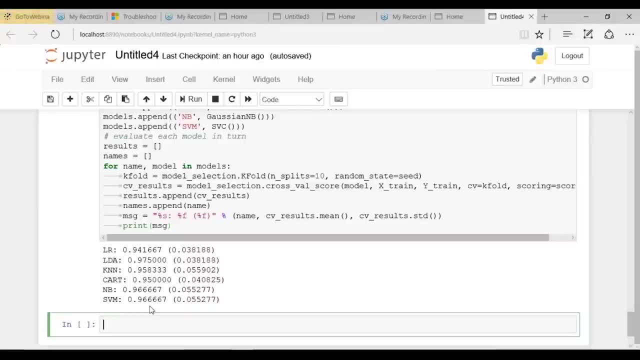 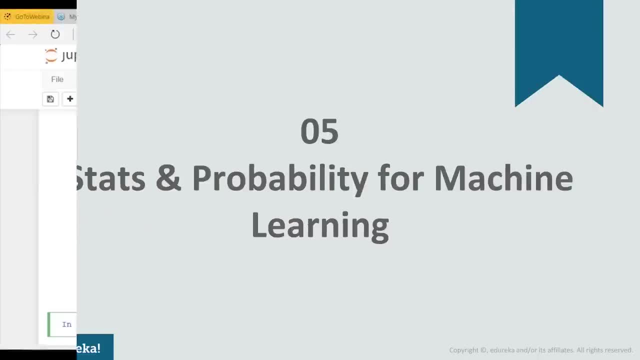 result: Okay, you can run the LDL model directly on the validation set and summarize the result as a final score, a confusion matrix and a classification report. Statistics and probability are essential because these disciples form the basic foundation Of all machine learning algorithms: deep learning, artificial. 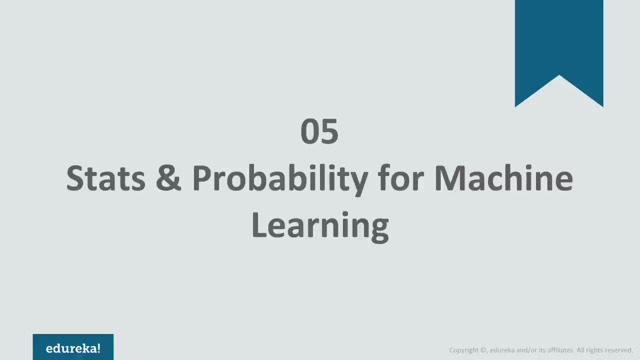 intelligence and data science. In fact, mathematics and probability is behind everything around us, from shapes, patterns and colors to the count of petals in a flower. mathematics is embedded in each and every aspect of our lives. So I'm going to go ahead and discuss the agenda for today with 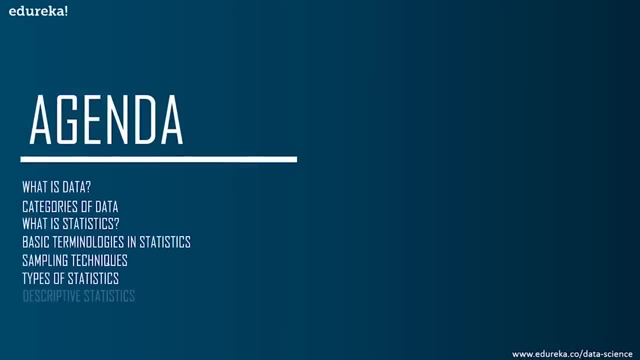 you all. We're going to begin the session by understanding What is data. After that we'll move on and look at the different categories of data, like quantitative and qualitative data. Then we'll discuss what exactly statistics is, the basic terminologies and statistics and a couple of sampling techniques. 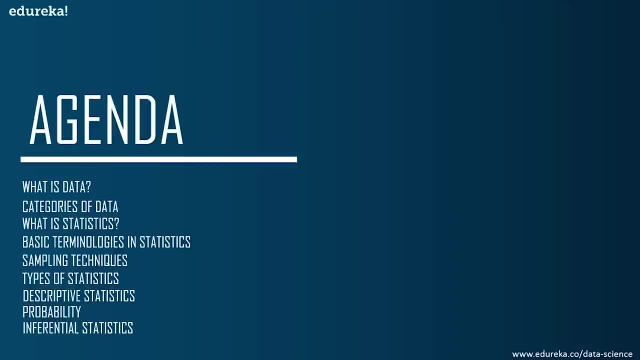 Once we're done with that, We'll discuss the different types of statistics, which involve descriptive and inferential statistics. then in the next session We'll mainly be focusing on descriptive statistics. here We'll understand the different measures of Center, measures of spread information. 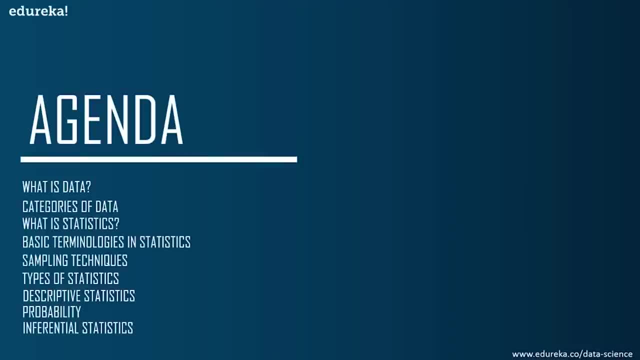 Gain and entropy. will also understand all of these measures with the help of a use case and, finally, will discuss what exactly a confusion Matrix is. once we've covered the entire descriptive statistics module, will discuss the probability module. here We'll understand what exactly probability is. the different 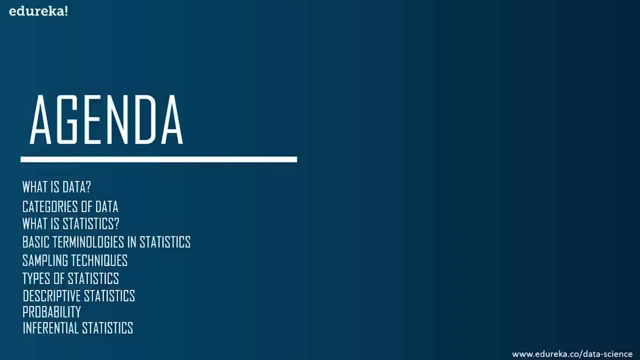 terminologies and probability, will also study the different probability distributions. Then we'll discuss the types of probability, which include marginal probability, joint and conditional probability. Then we'll move on and discuss a use case wherein we'll see examples that show us how the different types of probability 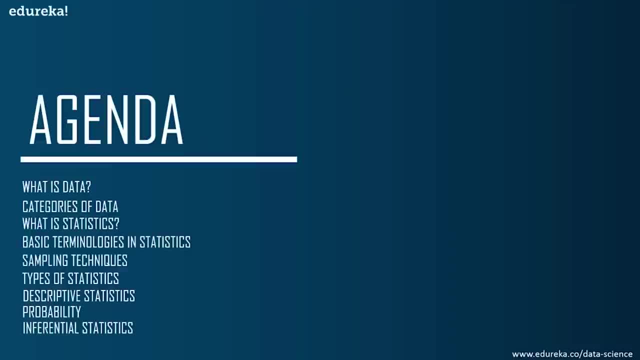 work and to better understand base theorem. We look at a small example. Also, I forgot to mention that at the end of the descriptive statistics module will be running a small demo in the R language. So for those of you who don't know much about our, I'll be explaining. 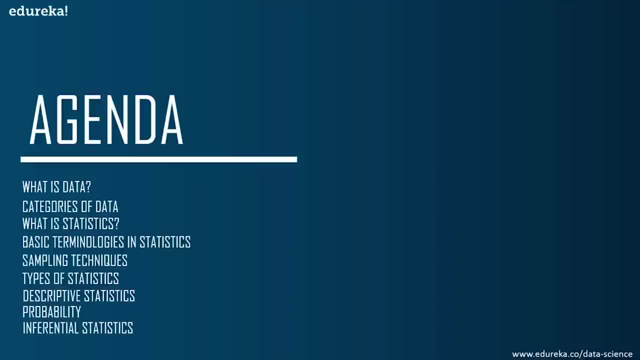 every line in depth, But if you want to have A more in-depth understanding about our, I'll leave a couple of blogs and a couple of videos in the description box. Y'all can definitely check out that content. now, after we've completed the probability module, will discuss the inferential. 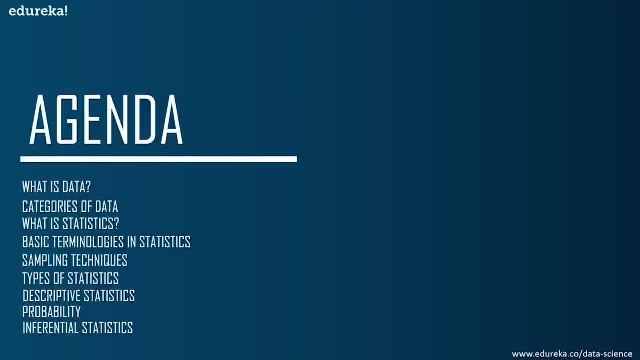 like quantitative and qualitative data. then we'll discuss what exactly statistics is, the basic terminologies and statistics and a couple of sampling techniques. Once we're done with that, we'll discuss the different types of statistics, which involve descriptive and inferential statistics. then in the next session, 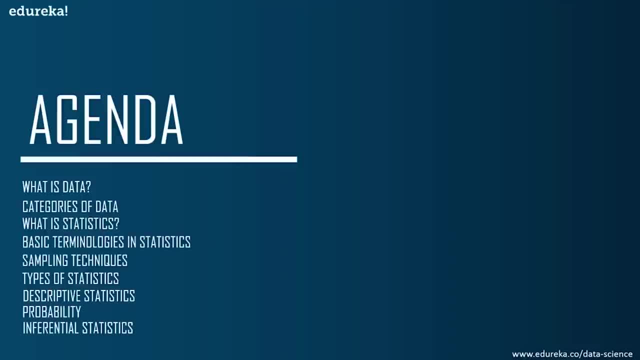 We'll mainly be focusing on descriptive statistics. here. We'll understand the different measures of Center, measures of spread, information gain and entropy will also understand all of these measures with the help of a use case. and finally, we'll discuss what exactly a confusion Matrix is once we've 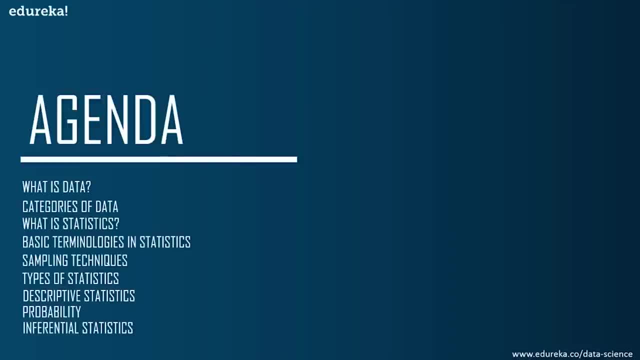 covered the entire descriptive statistics module. will discuss the probability module. here We'll understand what exactly probability is, the different terminologies and probability. will also study the different probability distributions. Then we'll discuss the types of probability, which include marginal probability, joint and conditional probability. 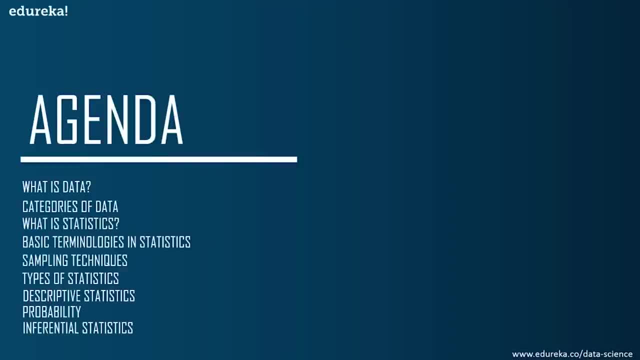 Then we'll move on and discuss a use case wherein we'll see examples that show us how the different types of probability work and to better understand base theorem. We look at a small example Also. I forgot to mention that at the end of the descriptive statistics. 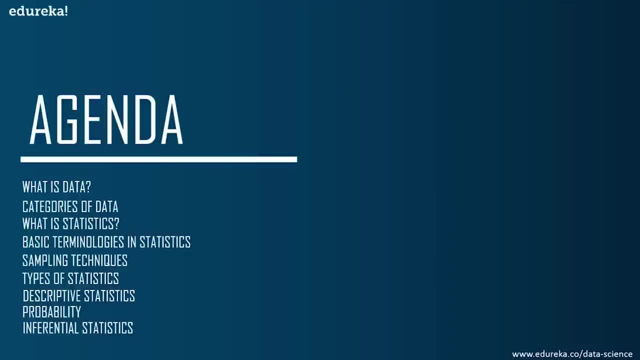 module will be running a small demo in the R language. So for those of you who don't know much about our, I'll be explaining every line in depth. But if you want to have a more in-depth understanding about our, I'll leave a couple of blogs and a couple of videos in the description. 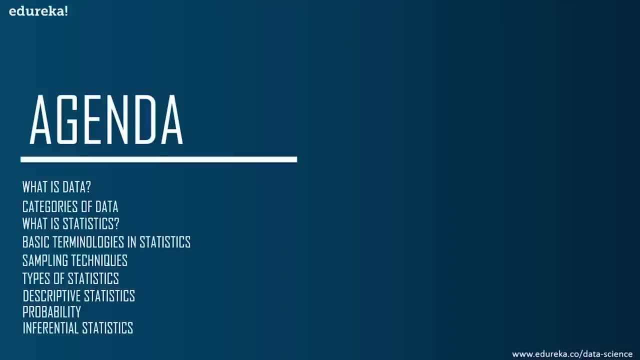 box. Y'all can definitely check out that content. now, after we've completed the probability module, will discuss the inferential statistics module. will start this module by understanding What is point estimation. will discuss what is confidence interval and how you can estimate the confidence interval. will also discuss 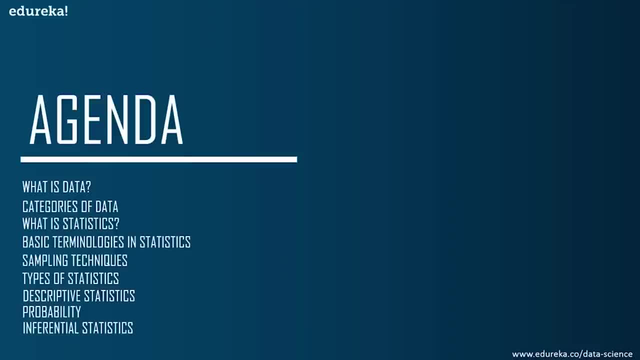 margin of error, and will understand all of these concepts by looking at a small use case. We'll finally And the inferential statistic module by looking at what hypothesis testing is. hypothesis Testing is a very important part of inferential statistics, So we'll end the session by looking at a use case that discusses 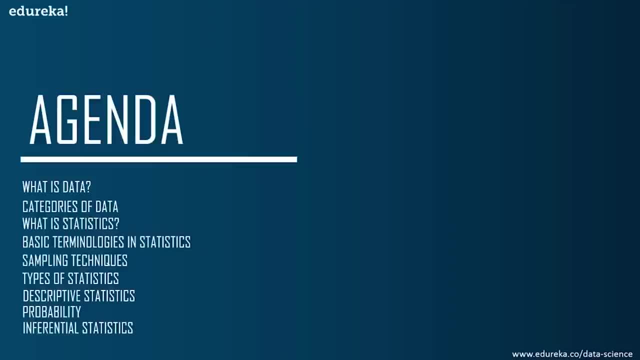 how hypothesis testing works. and, to sum everything up, We look at a demo that explains how inferential statistics works. All right, So, guys, there's a lot to cover today, So let's move ahead and take a look at our first topic, which is: 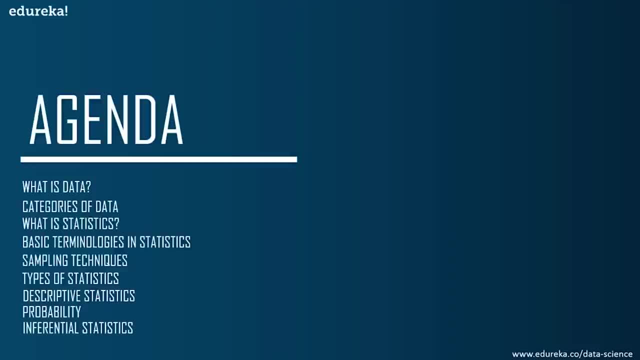 statistics module will start this module by understanding What is point estimation, will discuss what is confidence interval and how you can estimate the confidence interval. will also discuss margin of error and will understand all of these concepts by looking At a small use case. We finally end the inferential statistic module by looking at 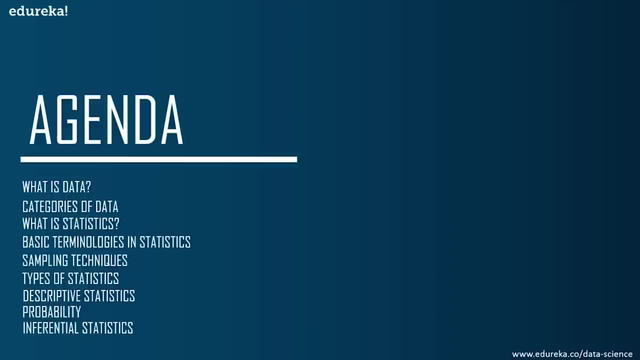 what hypothesis testing is. hypothesis testing is a very important part of inferential statistics, So we'll end the session by looking at a use case that discusses how hypothesis testing works and, to sum everything up, We look at a demo that explains how inferential statistics works. 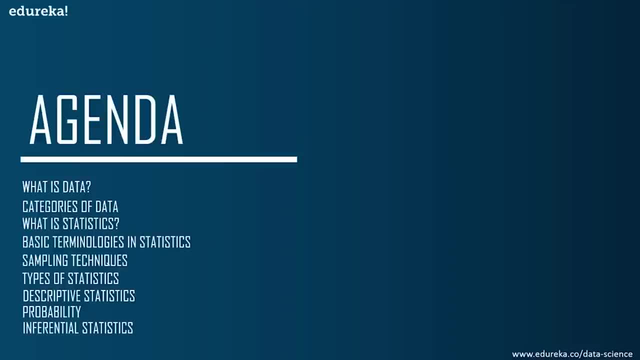 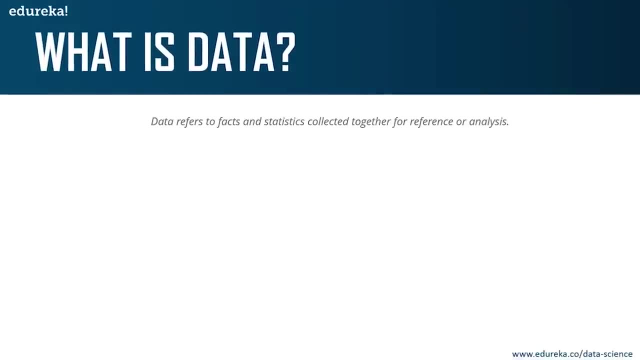 Alright. so, guys, there's a lot to cover today, So let's move ahead and take a look at our first topic, which is what is data? Now, this is a quite simple question. If I ask any of you, what is data? 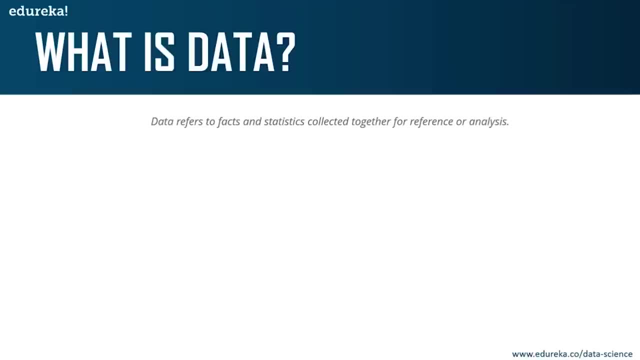 You'll see that it's a set of numbers or some sort of documents that I've stored in my computer. Now, data is actually everything. All right, look around you, There is data everywhere. Each click on your phone generates more data than you know. 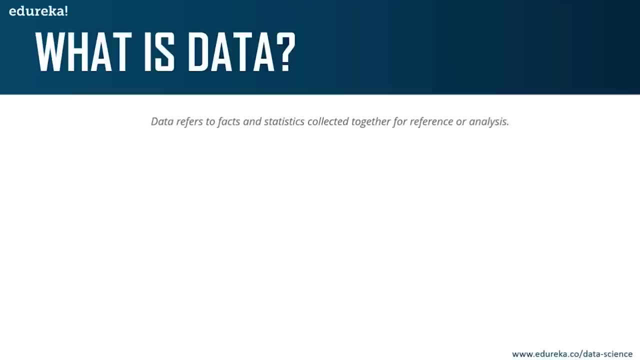 Now, this generated data provides insights for analysis and helps us make better business decisions. This is why data is so important to give, So a formal definition: data refers to facts and statistics collected together for reference or analysis. All right, This is the definition of data in terms of statistics and probability. 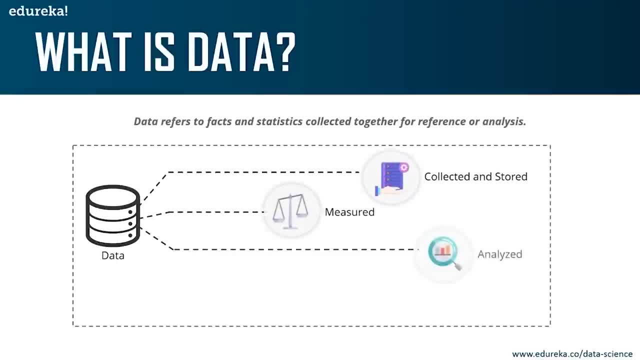 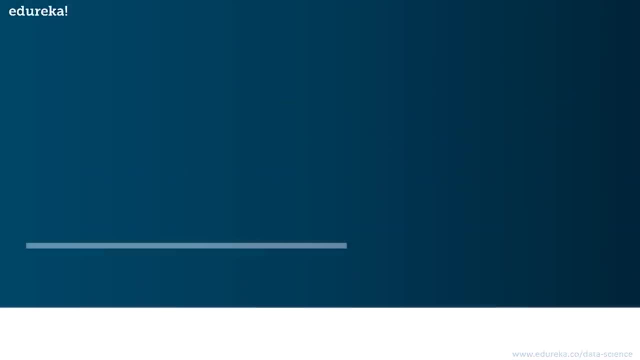 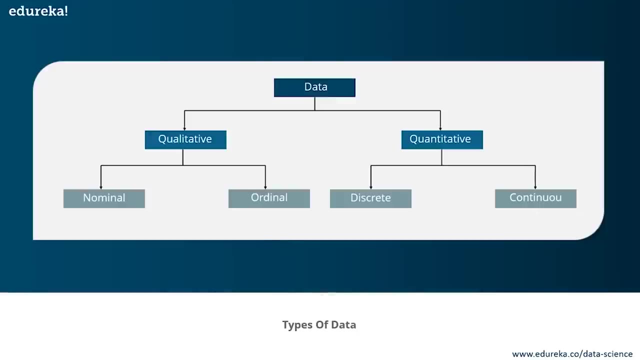 So, as we know, data can be collected, It can be measured and analyzed, It can be visualized by using statistical models and graphs. Now, data is divided into two major subcategories, All right. So first we have qualitative data and quantitative. These are the two different types of data under qualitative data, 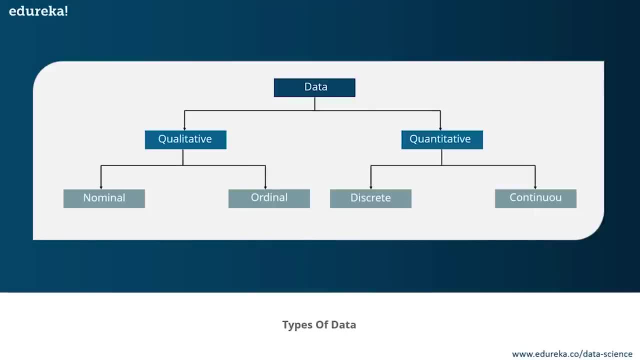 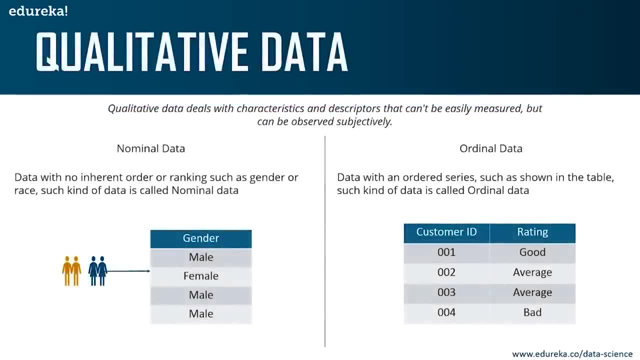 We have nominal and ordinal data, and under quantitative data, We have discrete and continuous data. Now let's focus on qualitative data. Now, this type of data deals with characteristics and descriptors that can't be easily measured, but can be observed subjectively. Now qualitative data is further divided into nominal and ordinal data. 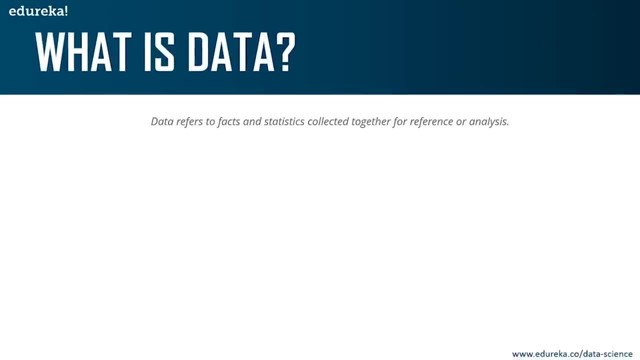 what is data? now, This is a quite simple question. If I ask any of you what is data, you'll see that it's a set of numbers or some sort of documents that I've stored in my computer. Now, data is actually everything. 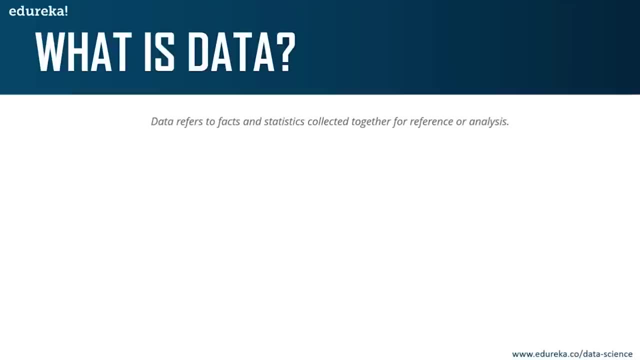 All right. look around you. There is data everywhere. Each click on your phone generates more data than you know Now. this generated data provides insights for analysis and helps us make better business decisions. This is why data is so important. to give you a formal definition: data. 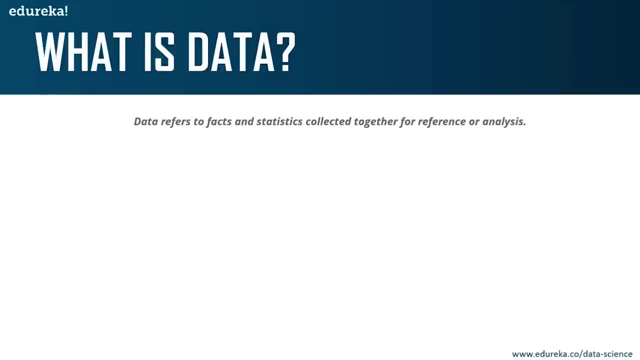 refers to facts And statistics collected together for reference or analysis. All right, This is the definition of data in terms of statistics and probability. So, as we know, data can be collected, It can be measured and analyzed. It can be visualized by using statistical models and graphs. 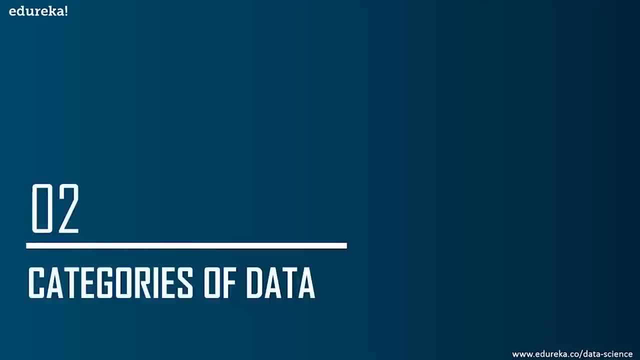 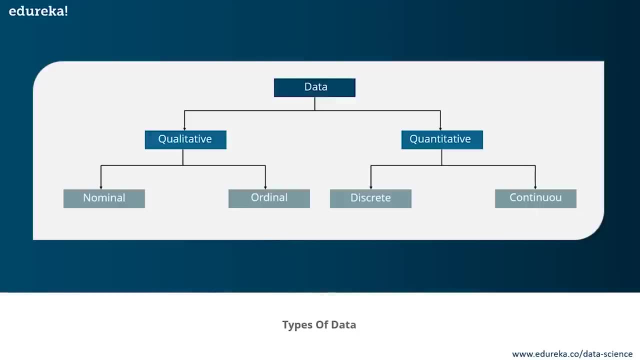 Now data is divided into two major subcategories. All right, So first we have qualitative data and quantitative data. These are the two different types of data. Under qualitative data We have nominal and ordinal data, and under quantitative data We have discrete and continuous data. 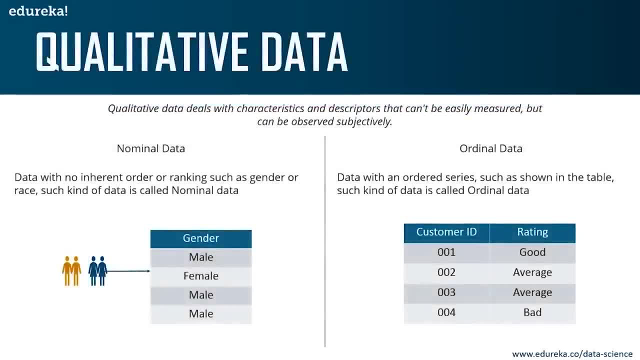 Now let's focus on qualitative data. Now, this type of data deals with characteristics and descriptors that can't be easily measured, but can be observed subjectively. Now qualitative data is further divided into nominal and ordinal data. So nominal data is any sort of data that doesn't have any order or 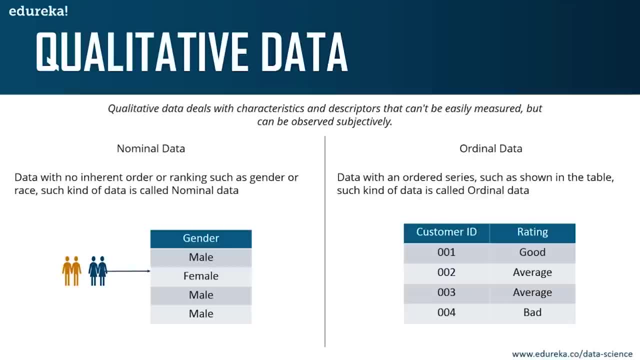 ranking. Okay, an example of nominal data is gender. Now, there is no ranking in gender. There's only male, female or other right. There is no one, two, three, four or any sort of ordering in gender. Race is another example of nominal data. 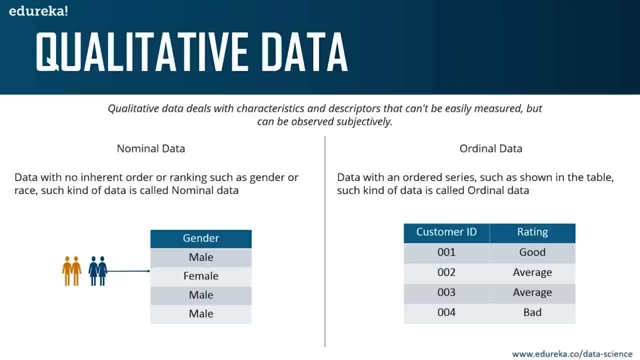 Now, ordinal data is basically an ordered series of information. Okay, let's say that you went to a restaurant. Okay, your information is stored in the form of customer ID, All right. So basically, you are represented With a customer ID. Now you would have rated their service as either good or average. 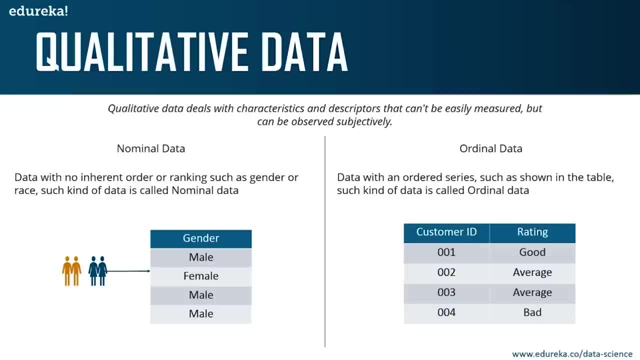 All right, that's how an ordinal data is, and similarly, they'll have a record of other customers who visit the restaurant, along with their ratings. All right, So any data which has some sort of sequence or some sort of order to it is known as ordinal data. 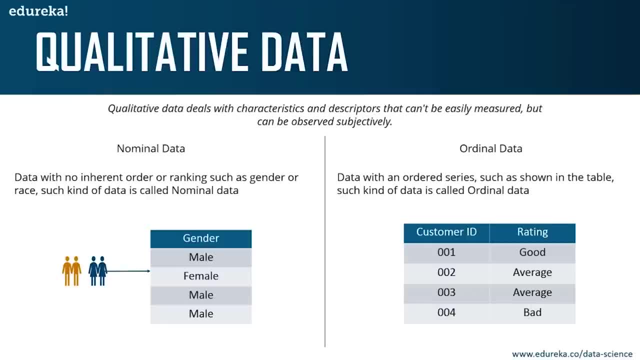 So nominal data is any sort Of data that doesn't have any order or ranking. Okay, an example of nominal data is gender. Now, there is no ranking in gender. There's only male, female or other right. There is no one, two, three, four or any sort of ordering in gender. 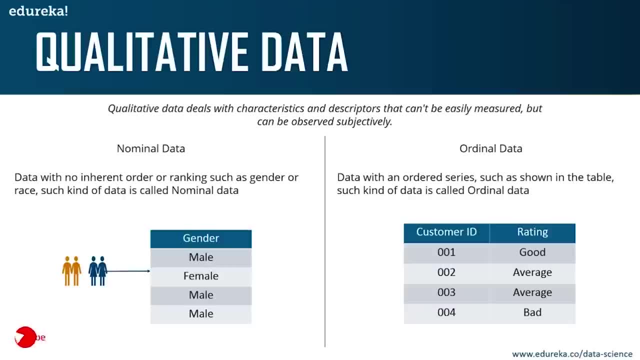 Race is another example of nominal data. Now, ordinal data is basically an ordered series of information. Okay, let's say that you went to a restaurant. Okay, your information is stored in the form of customer ID, All right, So basically, you are represented with a customer ID. 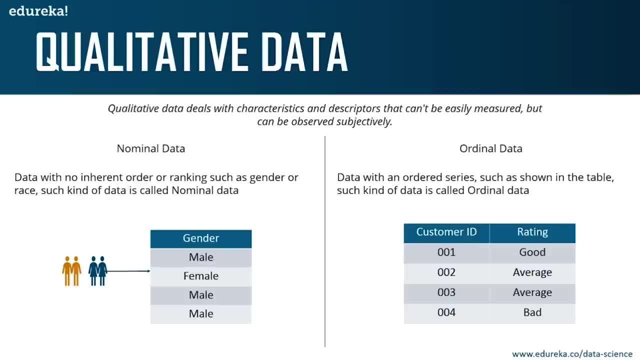 Now you would have rated their service as either good or average. All right, that's how an ordinal data is, And similarly, they'll have a record of other customers who visit the restaurant, along with their ratings. All right, So any data which has some sort of sequence or some sort of order to 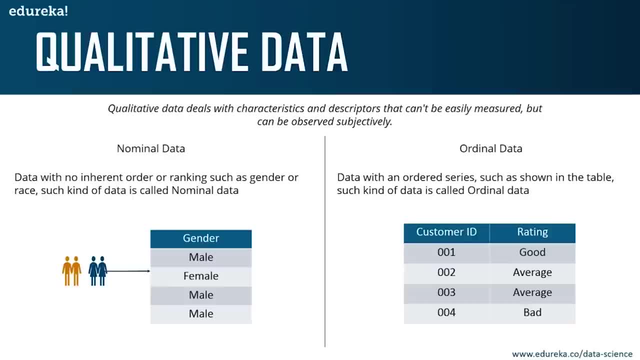 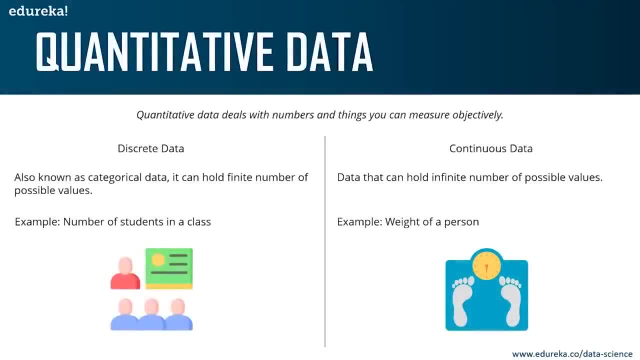 it is known as ordinal data. All right, So, guys, this is pretty simple to understand. Now let's move on And look at quantitative data. So quantitative data basically deals with numbers and things. Okay, you can understand that by the word quantitative itself. 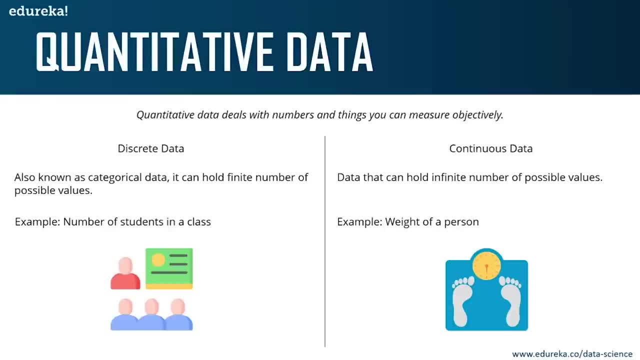 Quantitative is basically quantity, right, So it deals with numbers, It deals with anything that you can measure objectively. All right, So there are two types of quantitative data. There is discrete and continuous data. Now, discrete data is also known as categorical data, and it can hold a 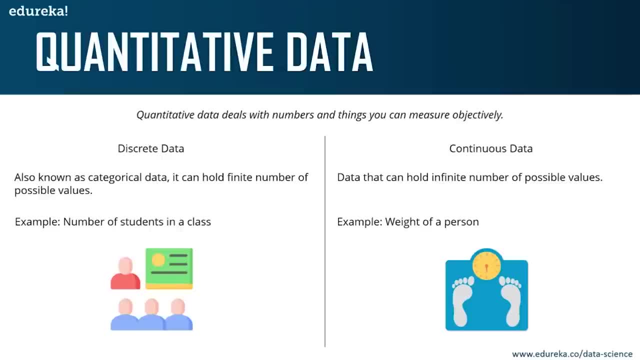 finite number of possible values. Now, the number of students in a class is a finite number. All right, you can't have infinite number of students in a class. Let's say in your fifth grade there were hundred students in your class. All right, there weren't infinite number, but there was a definite finite. 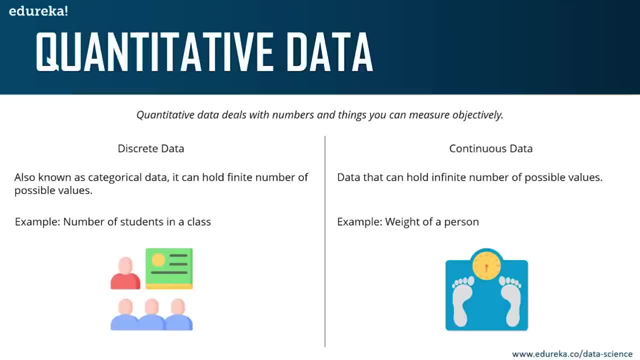 number of students in your class. Okay, that's discrete data. Next, we have continuous data. Now, this type of data can hold infinite number of possible values, Okay. So when you say weight of a person is an example of continuous data, what I mean to say is my weight can be 50 kgs, or it can be 50.1 kgs, or 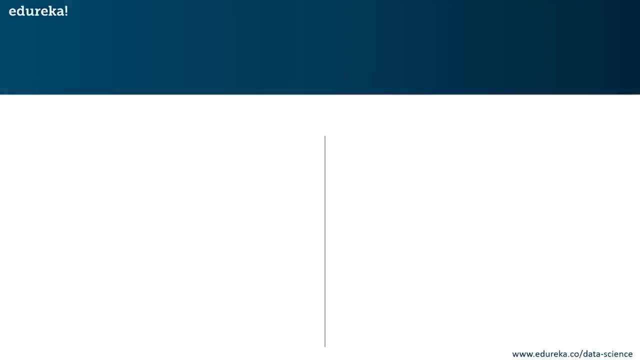 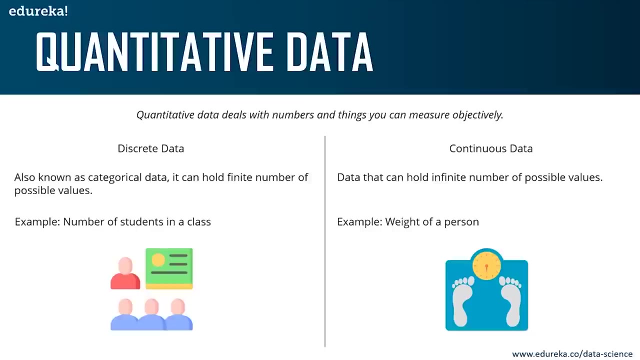 All right. So, guys, this is pretty simple to understand. Now let's move on and look at quantitative data. So quantitative Data basically deals with numbers and things. Okay, you can understand that by the word quantitative itself. quantitative is basically quantity, right? 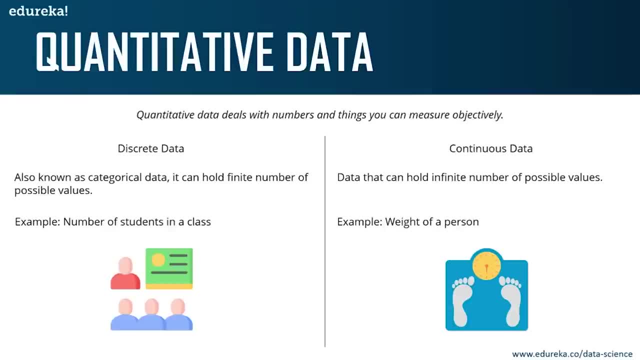 So it deals with numbers. It deals with anything that you can measure objectively. All right, So there are two types of quantitative data. There is discrete and continuous data. Now, discrete data is also known as categorical data, and it can hold a finite number of possible values. 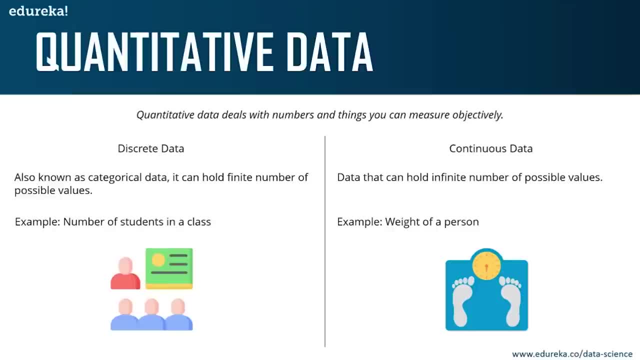 Now, the number of students In a class is a finite number. All right, you can't have infinite number of students in a class. Let's say in your fifth grade There were hundred students in your class. All right, there weren't infinite number, but there was a definite. 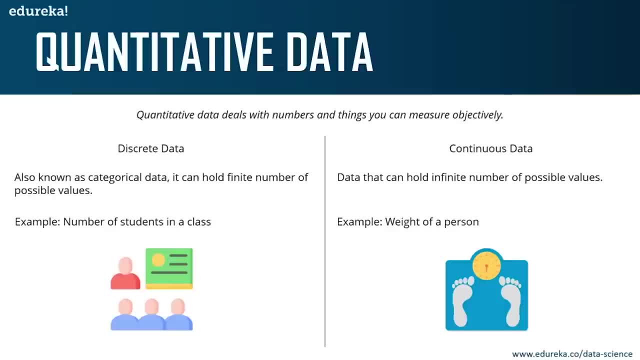 finite number of students in your class. Okay, that's discrete data. Next, we have continuous data. Now, this type of data can hold infinite number of possible values. Okay. So when you say, weight of a person is an example of continuous data. 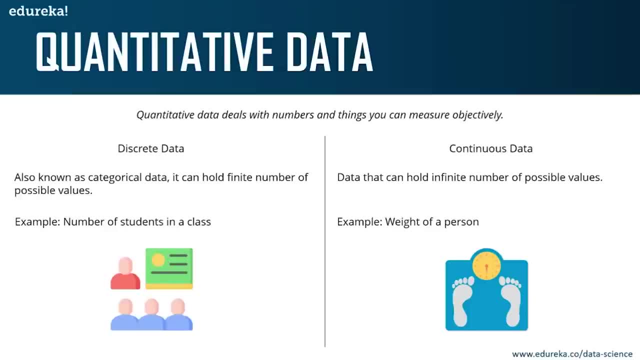 What I mean to say is: my weight can be 50. TKGs, or it can be 50.1 kgs, or it can be 50.001 kgs or 50.0001 or 50.023 and so on. right, there are infinite number of possible values, right? 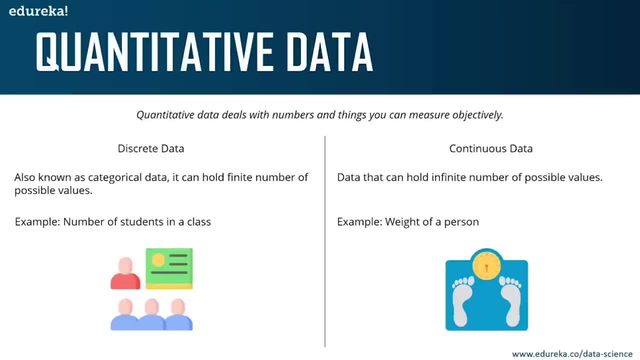 So this is what I mean by continuous data. All right, This is the difference between discrete and continuous data, And also I like to mention a few other things over here. Now, there are a couple of types of data, Variables as well. 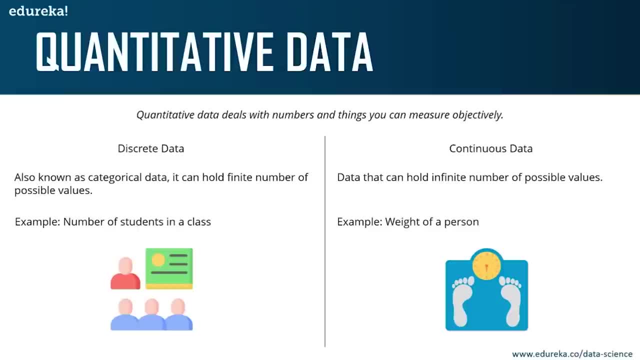 All right, we have a discrete variable and we have a continuous variable. discrete variable is also known as a categorical variable. All right, it can hold values of different categories. Let's say that you have a variable called message and there are two types of values that this variable can hold. 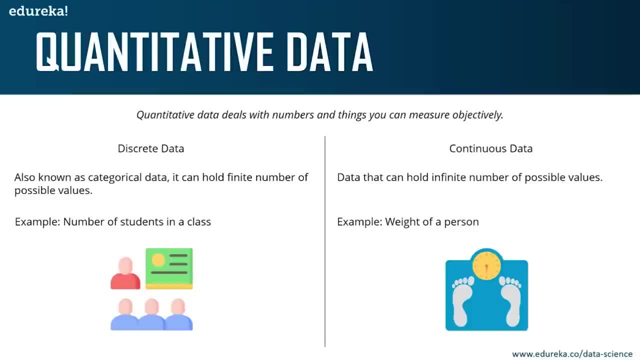 Let's say that your message can either be a spam message or a non-spam message. Okay, that's when you call a variable as discrete or categorical. Categorical variable: All right, because it can hold values that represent different categories of data. 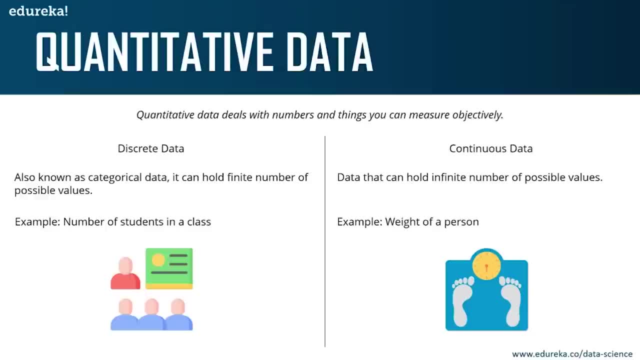 it can be 50.001 kgs or 50.0001 or 50.023 and so on. right, There are infinite number of possible values, right? So this is what I mean by continuous data. All right, This is the difference between discrete and continuous data, and also I like 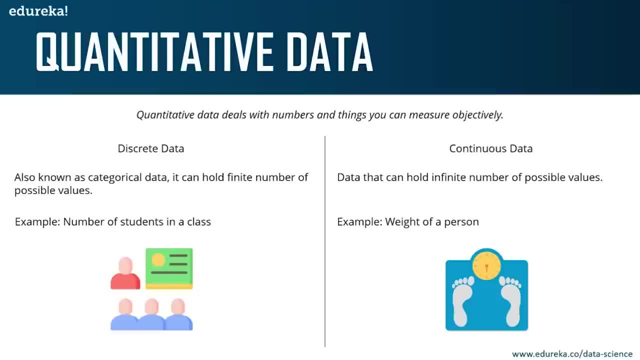 to mention a few things. You other things over here. Now there are a couple of types of variables as well. All right, we have a discrete variable and we have a continuous variable. discrete variable is also known as a categorical variable. All right, it can hold values of different categories. 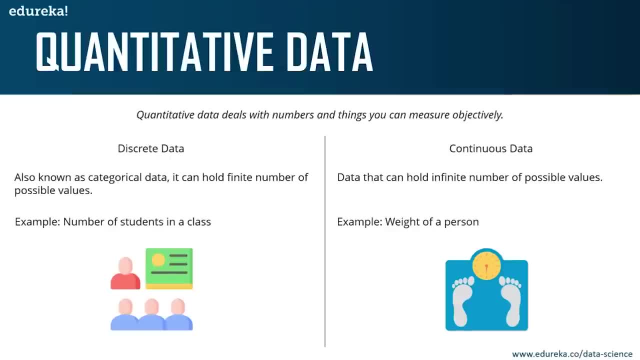 Let's say that you have a variable called message and there are two types of values that this variable can hold. Let's say that your message can either be a spam message or a non spam message. Okay, that's when you call a variable as discrete or categorical variable. 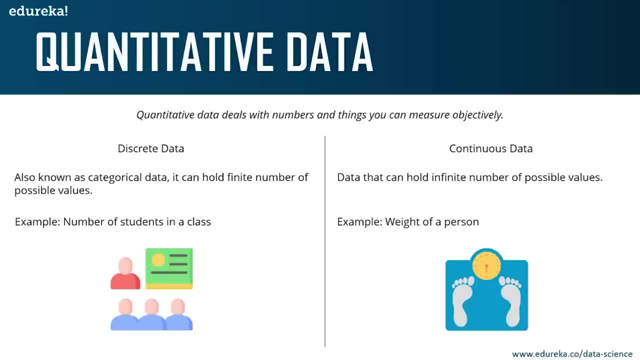 All right, because it can hold values that represent different categories of data. Now, continuous variables are basically variables that can store infinite number of values. So the weight of a person can be denoted as a continuous variable. All right, let's say there is a variable called weight and it can store 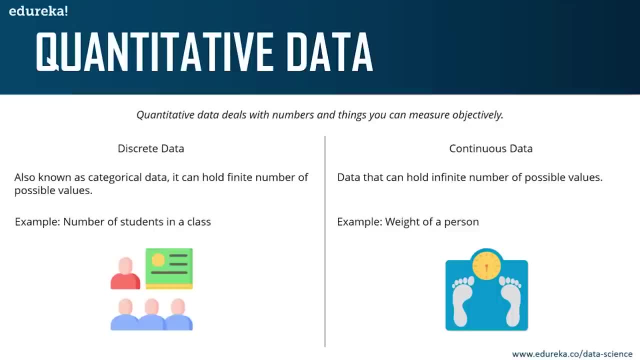 infinite number of possible values. That's why we'll call it a continuous variable. So, guys, basically, variable Is anything that can store a value, right? So if you associate any sort of data with a variable, then it will become either discrete variable or continuous variable. that is also dependent. 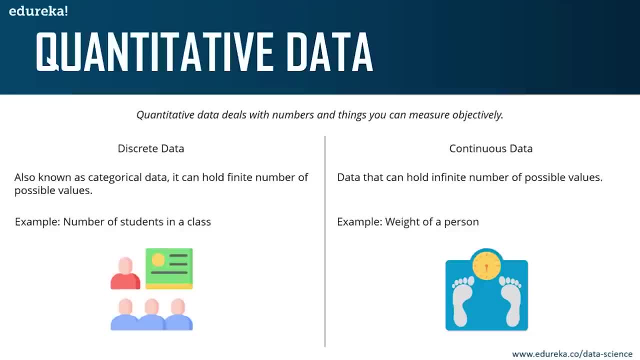 and independent type of variables. Now we won't discuss all of that in depth, because that's pretty understandable. I'm sure all of you know what is independent variable and dependent variable. right, dependent variable is any variable whose value depends on any other independent variable. 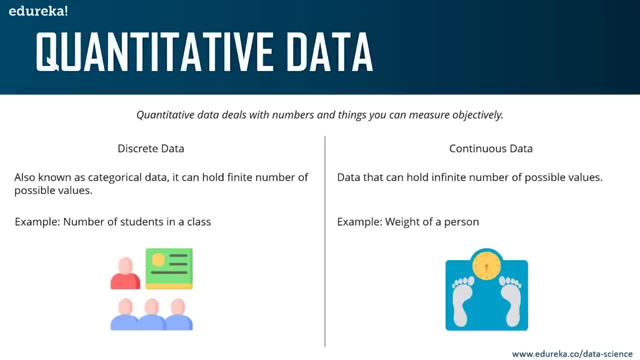 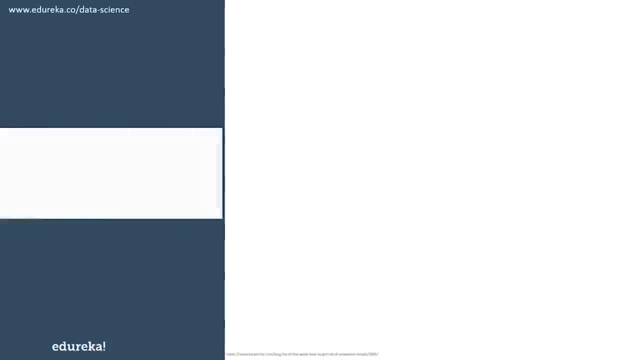 So, guys, that much knowledge I expect all of you to have, all right. So now let's move on and look at our next topic, which is: what is statistics? now coming to the formal definition of statistics: statistics is an area of applied mathematics which is concerned with data. 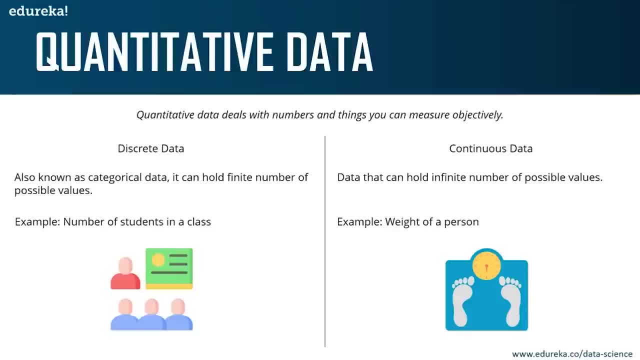 Now, continuous variables are basically variables that can store infinite number of values. So the weight of a person can be denoted as a continuous variable. All right, let's say there is a variable called weight and it can store infinite number of possible values. 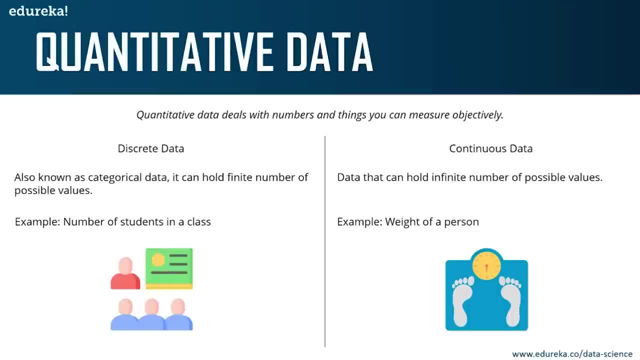 That's why we'll call it a continuous variable. So, guys, basically variable is anything that can store a value, right? So if you associate any sort of data with a variable, then it will become either discrete variable or continuous variable. that is also dependent and independent type of. 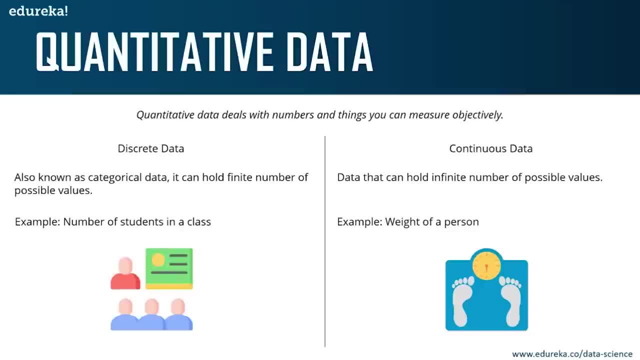 variables. Now we won't discuss all of that in depth, because that's pretty understandable. I'm sure all of you know what is independent variable and dependent variable, right? Dependent variable is any variable whose value depends on any other independent variable. 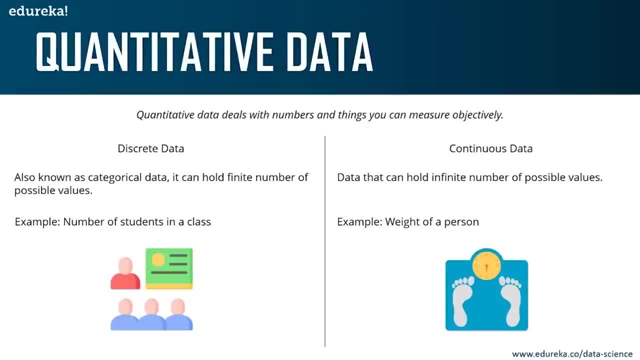 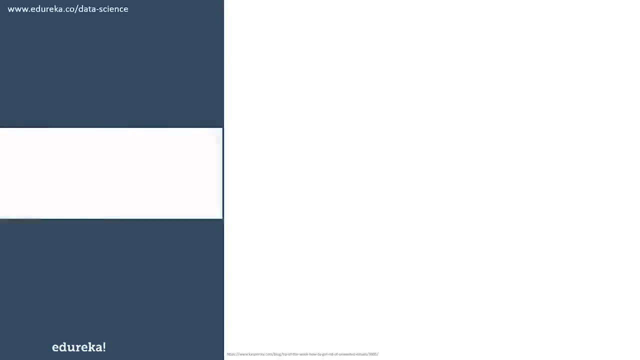 So, guys, that much knowledge I expect all of you to have, All right. So now let's move on and look At our next topic, which is: what is statistics? Now coming to the formal definition of statistics: statistics is an area of applied mathematics which is concerned with data collection. 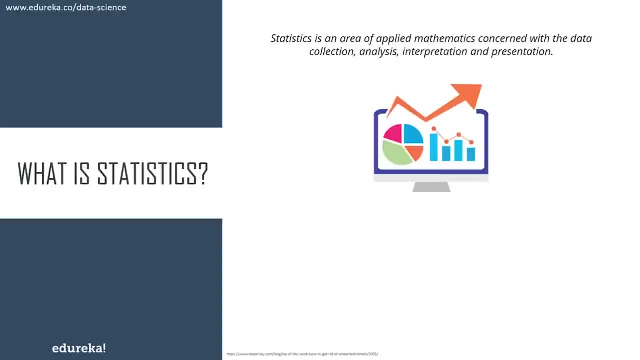 analysis, interpretation and presentation. Now, usually when I speak about statistics, people think statistics is all about analysis. but statistics has other parts to it. It has data collection is also a part of statistics. data interpretation, presentation, visualization- all of this comes into statistics. 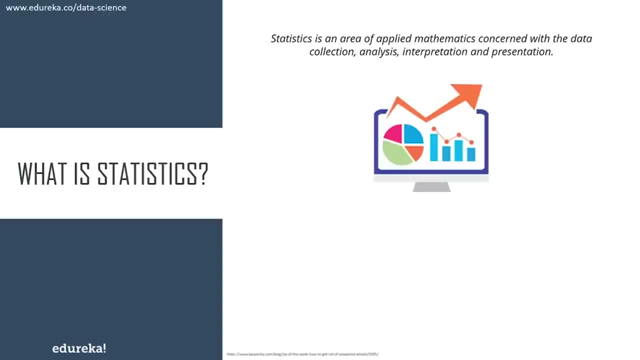 All right, You're going to use statistical methods to visualize data, to collect data, to interpret data, All right. So the area of mathematics deals with understanding how data can be used to solve complex problems. Okay, Now I'll give you a couple of examples that can be solved by using. 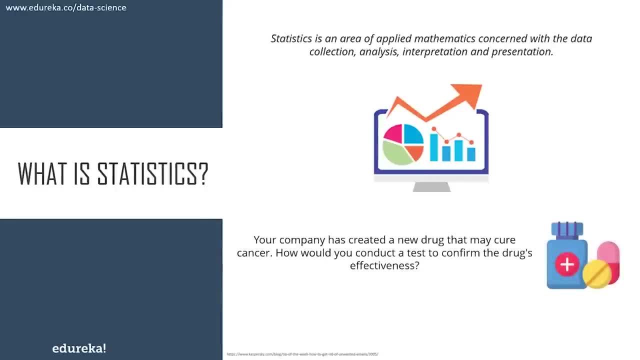 statistics. Okay, Let's say that your company has created a new drug that make your cancer. How would you conduct Test to confirm the drugs effectiveness? Now, even though this sounds like a biology problem, this can be solved with statistics. All right, you will have to create a test which can confirm the 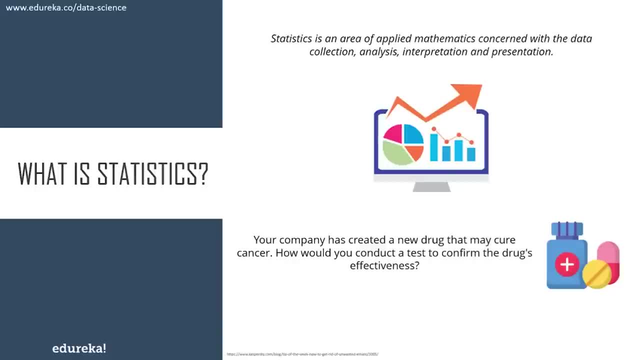 effectiveness of the drug. All right, This is a common problem that can be solved using statistics. Let me give you another example. You and a friend are at a baseball game and, out of the blue, he offers you a bet that neither team will hit a home run in that game. 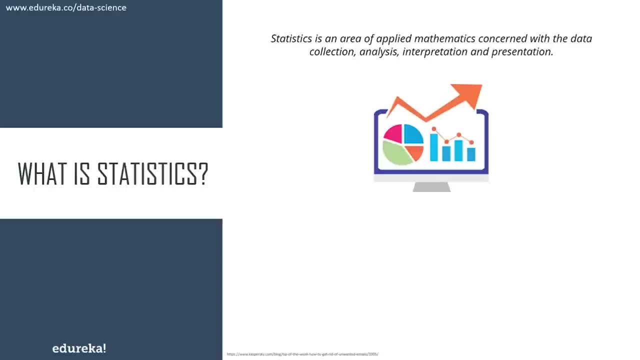 collection, analysis, interpretation and presentation. Now, usually when I speak about statistics, people think statistics is all about analysis. but statistics has other parts to it. It has data. Data collection is also a part of statistics. data interpretation, presentation, visualization- All of this comes into statistics. 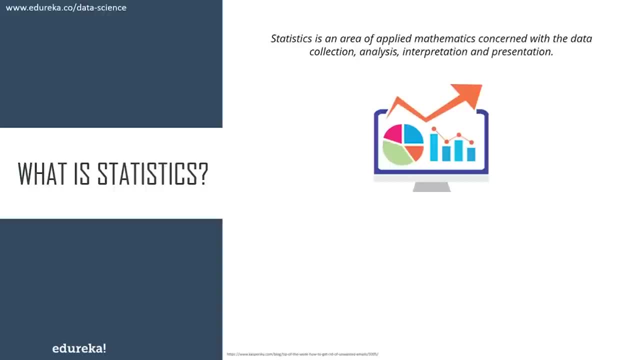 All right, you're going to use statistical methods to visualize data, to collect data, to interpret data, All right. So the area of mathematics deals with understanding how data can be used to solve complex problems. Okay, Now I'll give you a couple of examples that can be solved by using. 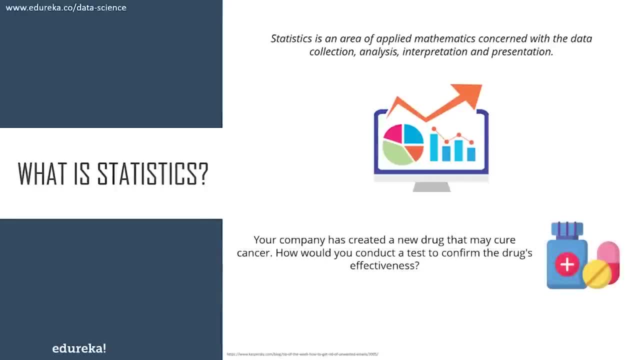 statistics. Okay, let's say that your company has created a new Drug that make your cancer. How would you conduct a test to confirm the drugs effectiveness? Now, even though this sounds like a biology problem at this, can be solved with statistics. 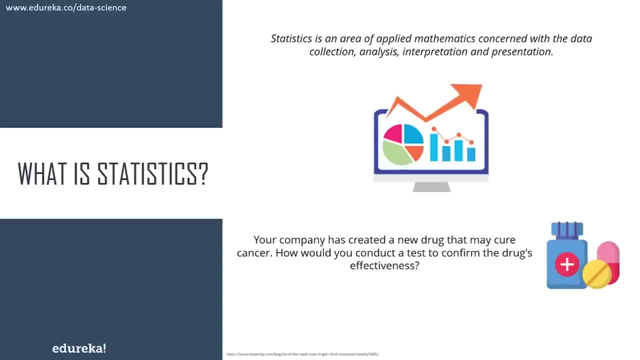 All right, you will have to create a test which can confirm the effectiveness of the drug. All right, This is a common problem that can be solved using statistics. Let me give you another example. you and a friend are at a baseball game and, out of the blue, he offers you a bet that neither team will. 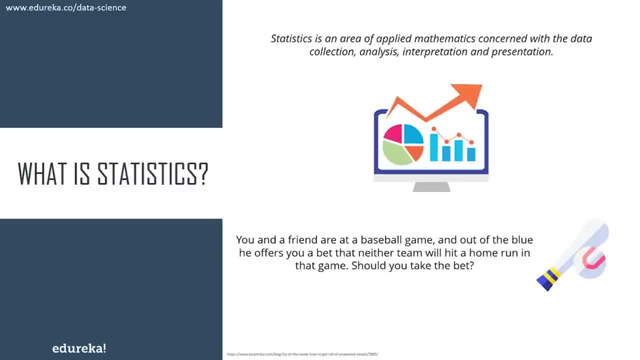 hit a home run in that game, Should you take the bet? All right. here You just discuss the probability of whether you'll win or lose. All right, This is another problem that comes under statistics. Let's look at another example. The latest sales data has just come in and your boss wants you to. 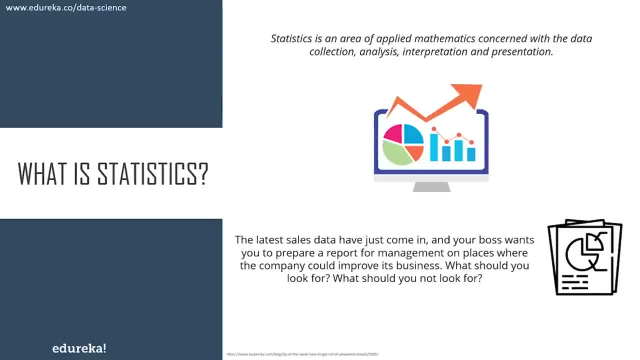 prepare a report for management on places where the company could improve its business. What should you look for And what should you not look for now? This problem involves a lot of data analysis. We'll have to look at the different variables that are causing your 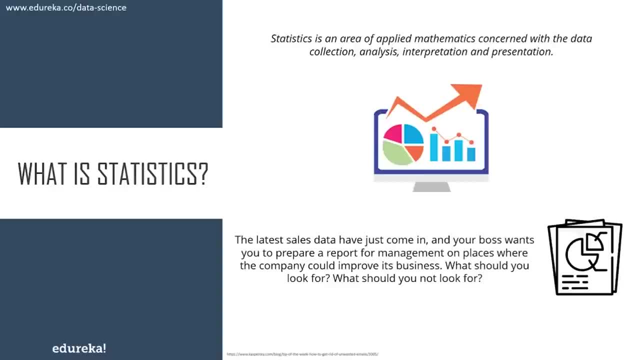 business to go down, or that you have to look at a few variables that are increasing the performance of your models and does growing your business All right. So this involves a lot of data analysis, and the basic idea behind data analysis is to use statistical techniques in order to figure out the 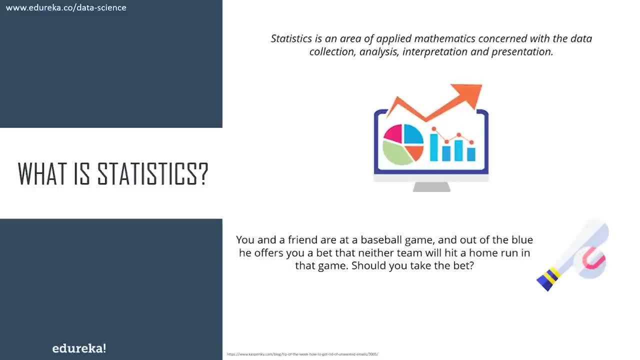 Should you take the bet? All right. Here you just discuss the probability of whether you'll win or lose. All right, This is another problem that comes under statistics. Let's look at another example. The latest sales data has just come in and your boss wants you to. 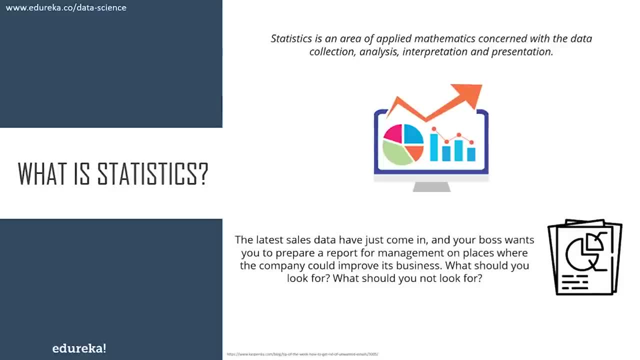 prepare a report for management on places where the company could improve its business. What should you look for And what should you not look for? Now? this problem involves a lot of data analysis. We'll have to look at the different variables that are causing your 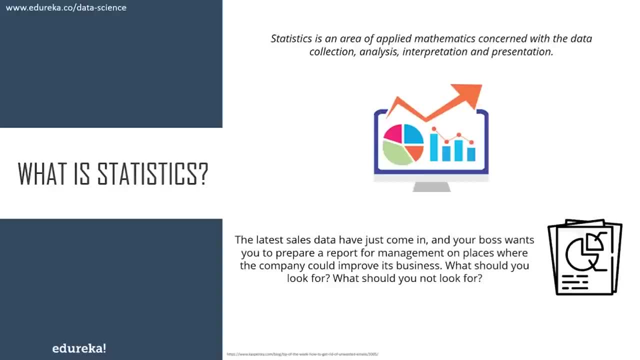 business to go down, Or you have to look at a few variables that are increasing the performance of your models and thus growing your business. All right, So this involves a lot of data analysis, and the basic idea behind data analysis is to use statistical techniques in order to figure out the 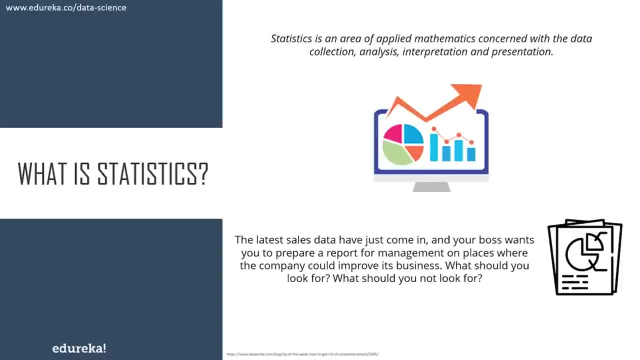 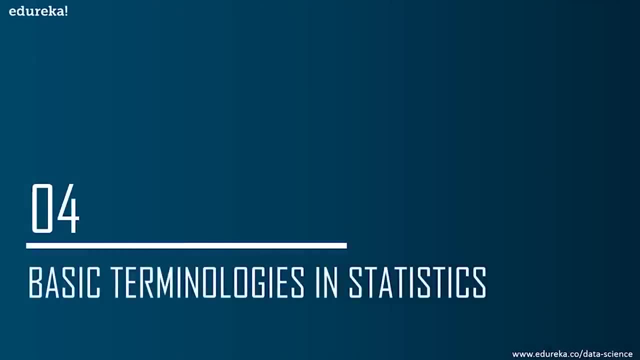 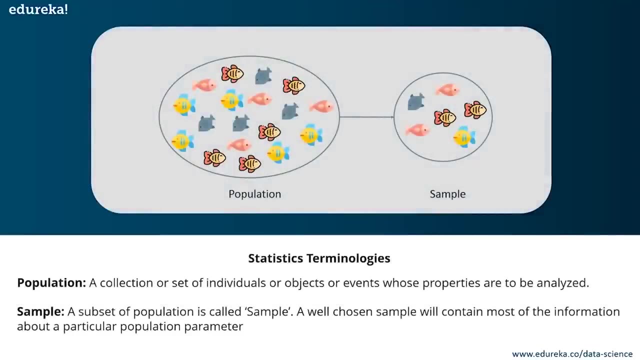 relationship between different variables or different components in your business. Okay, So now let's move on and look at our next topic, which is basic terminologies in statistics. Now, before you dive deep Into statistics, it is important that you understand basic terminologies. 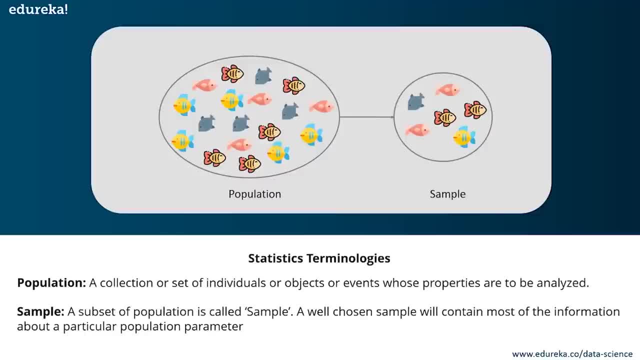 used in statistics. The two most important terminologies in statistics are population and sample. So throughout the statistics course, or throughout any problem that you're trying to solve with statistics, you will come across these two words, which is population and sample. Now, population is a collection or a set of individuals or objects, or 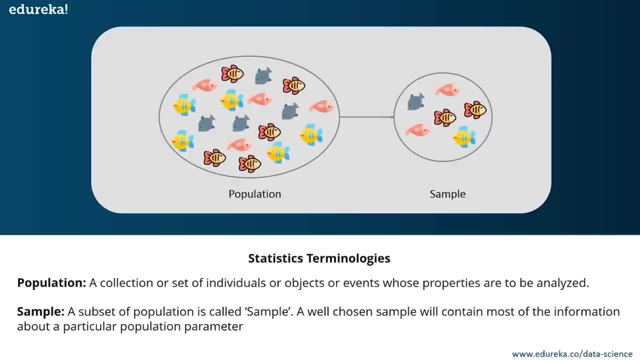 events whose properties are to be Analyzed. Okay, so basically, you can refer to population as a subject that you're trying to analyze. Now, a sample is just like the word suggests: It's a subset of the population. So you have to make sure that you choose the sample in such a way that 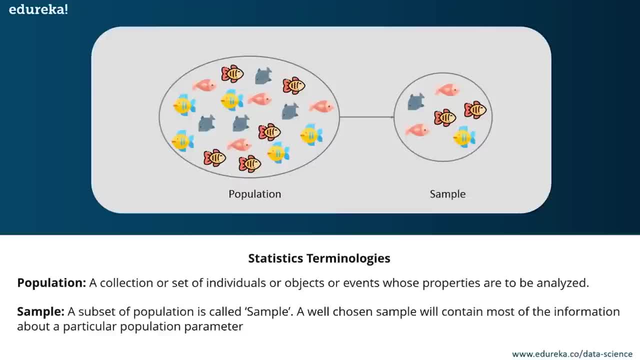 it represents the entire population, All right. it shouldn't focus at one part of the population. Instead, it should represent the entire population. That's how your sample should be chosen, So a well-chosen sample will contain Most of the information about a particular population parameter. 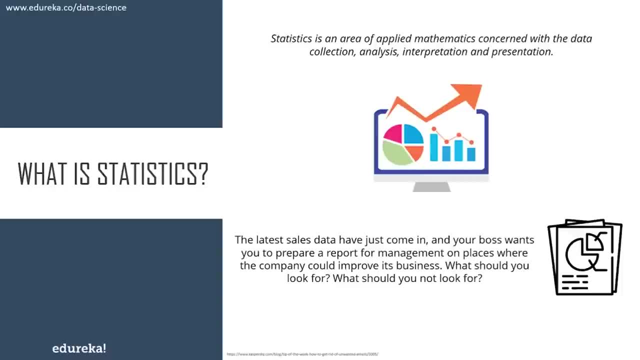 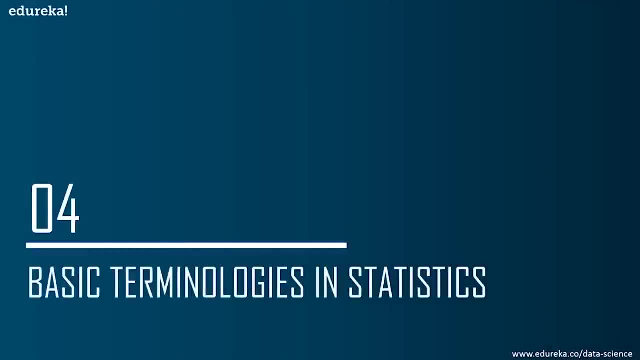 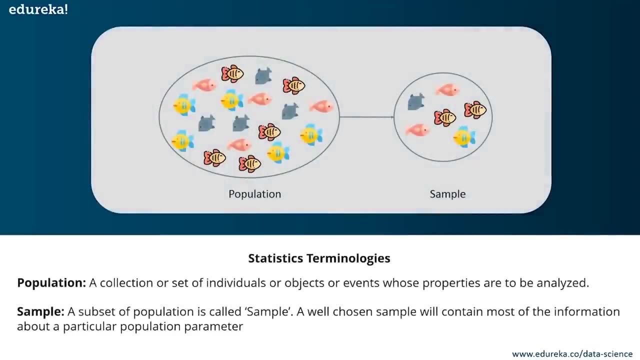 relationship between different variables or different components in your business. Okay, so now let's move on and look at our next topic, which is basic terminologies in statistics. Now, before you dive deep into statistics, it is important that you understand basic terminologies used in statistics. 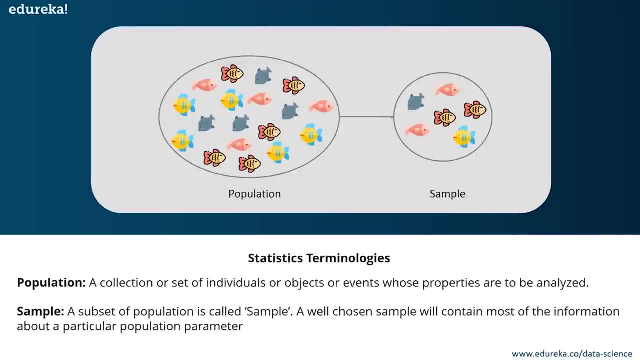 The two most important terminologies in statistics are population and sample. So throughout the statistics course, or throughout any problem that you're trying to solve with statistics, you will come across these two words, which is population and sample. Now, population is a collection or a set. 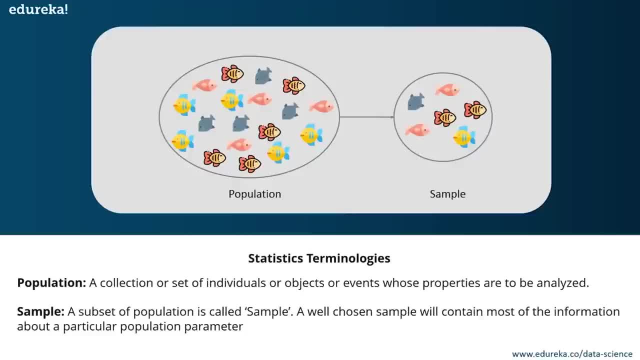 Of individuals or objects or events whose properties are to be analyzed. Okay, so basically, you can refer to population as a subject that you're trying to analyze Now. a sample is just like the word suggests: It's a subset of the population. So you have to make sure that you choose the sample in such a way that 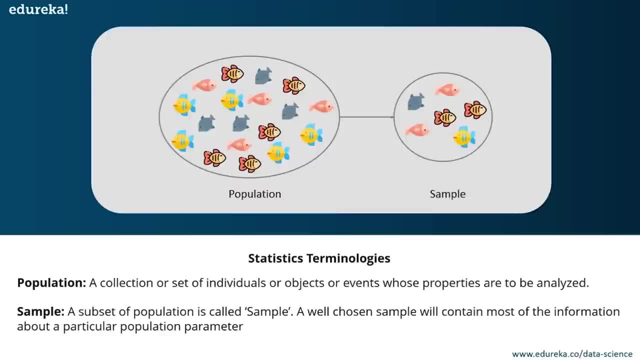 it represents the entire population, All right. It shouldn't focus at one part of the population. Instead, it should represent the entire population. That's how your sample should be chosen, So a well-chosen sample will contain most of the information about a 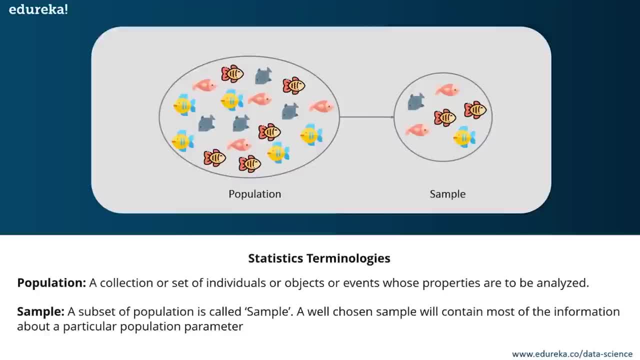 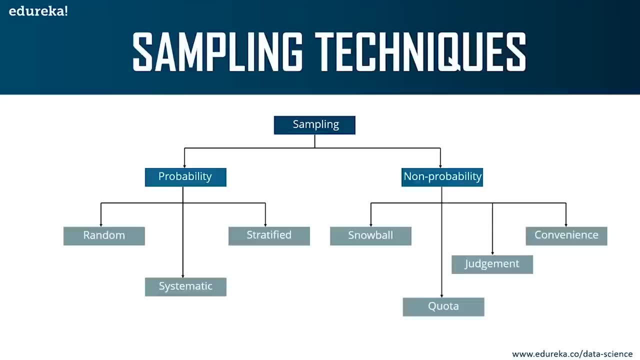 particular population parameter. Now you must be wondering how can one choose a sample that best represents the entire population? Now, sampling is a statistical method that deals with the selection of individual observations within a population. So sampling is performed in order to infer statistical knowledge about. 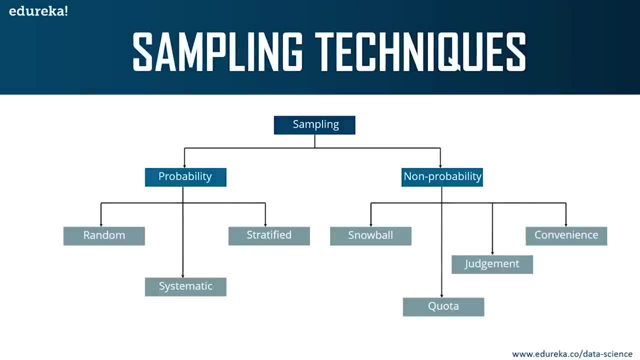 a population. All right, if you want to understand the difference between the two, then you can do that If you know the different statistics of a population, like the mean, the median, the mode or the standard deviation or the variance of a population. 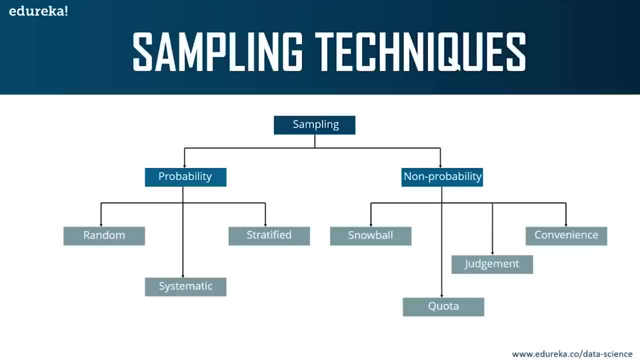 then you're going to perform sampling. All right, because it's not reasonable for you to study a large population and find out the mean median and everything else. So why is sampling performed? You might ask: what is the point of sampling? 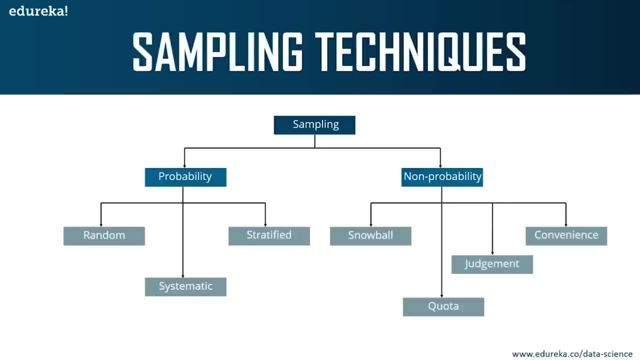 We can just study the entire population. Now, guys, think of a scenario wherein you're asked to perform a survey about the eating habits of teenagers In the US. So at present there are over 42 million teens in the US and this number is growing as we are speaking. 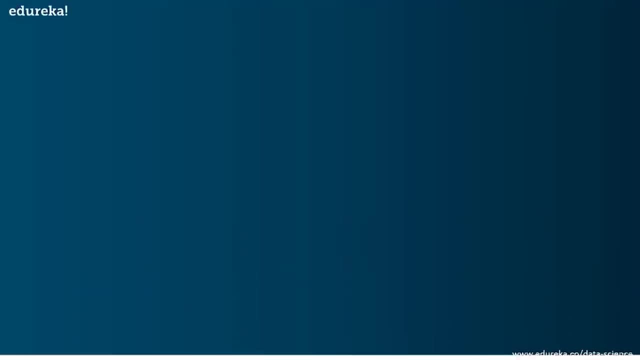 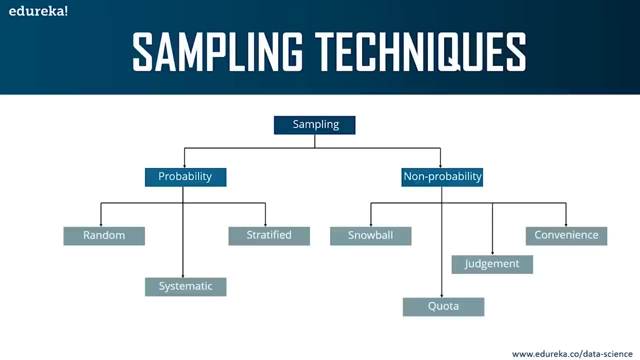 Now you must be wondering how can one choose a sample that best represents the entire population? Now, sampling is a statistical method that deals with the selection of individual observations within a population. So sampling is performed in order to infer statistical knowledge about a population. 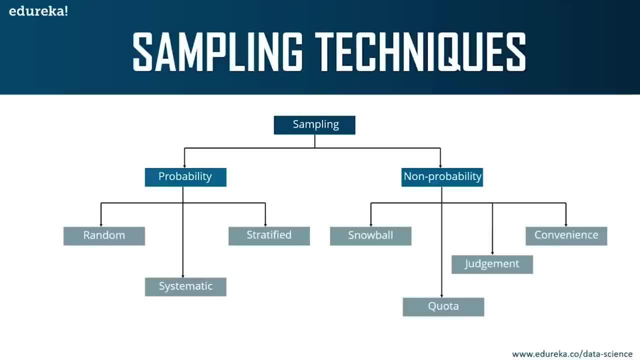 All right. if you want to understand the different statistics of a population, like the mean, the median, the mode or the Standard deviation or the variance of a population, then you're going to perform sampling, All right, because it's not reasonable for you to study a large population. 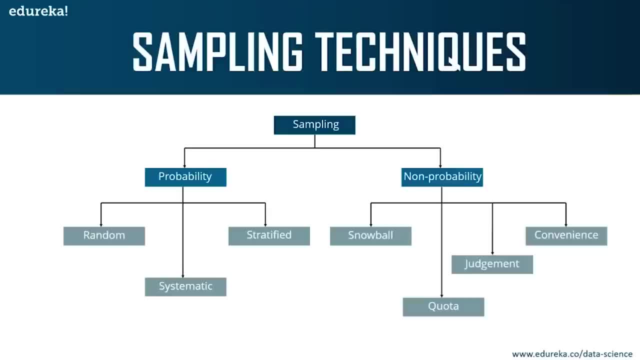 and find out the mean, median and everything else. So why is sampling performed? You might ask. what is the point of sampling? We can just study the entire population. Now, guys, think of a scenario wherein you're asked to perform a survey. 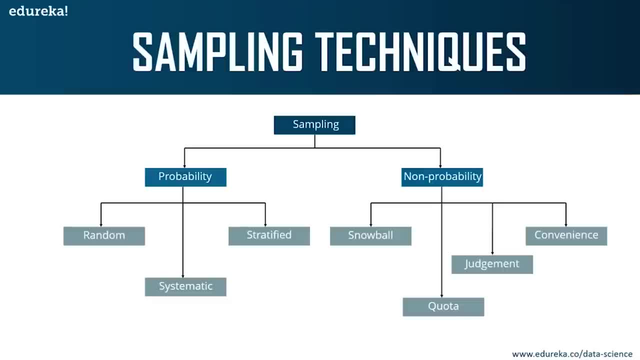 about the eating habits of teenagers in the US. So at present there are over 42 million Teens in the US and this number is growing as we are speaking right now, correct? Is it possible to survey each of these 42 million individuals about? 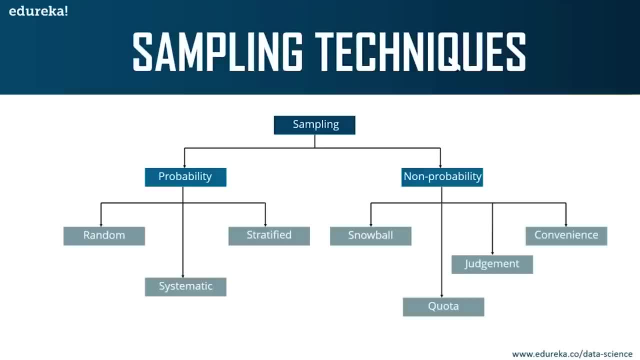 their health. Is it possible? Well, it might be possible, but this will take forever to do. Now, obviously it's not. it's not reasonable to go around knocking each door and asking for what does your teenage son eat? and all of that. 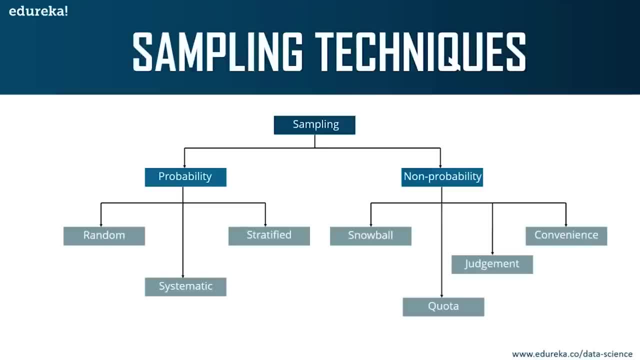 All right, this is not very reasonable. That's why sampling is used. It's a method wherein a sample of the population Is studied in order to draw inference about the entire population, So it's basically a shortcut to studying the entire population. 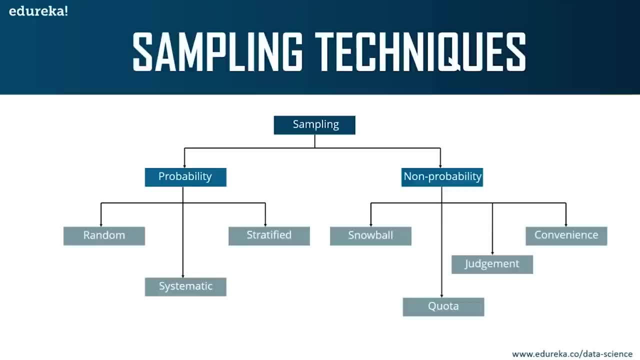 Instead of taking the entire population and finding out all the solutions, You're just going to take a part of the population that represents the entire population, and you're going to perform all your statistical analysis, your inferential statistics, on that small sample, All right, and that sample basically represents the entire population. 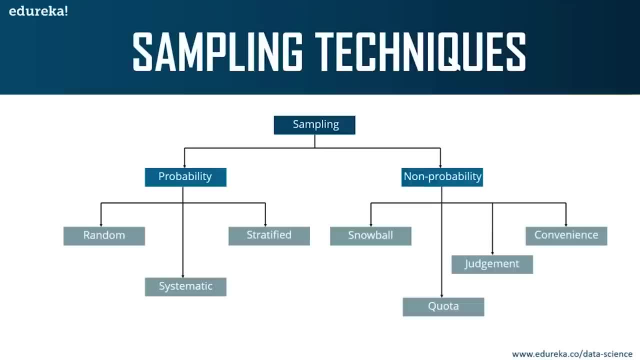 All right, So I'm sure I've made this clear to all: what is sample and what is population. Now there are two main types of sampling techniques that I'll discuss today. We have probability sampling and non-probability sampling. Now, in this video, we'll only be focusing on probability sampling. 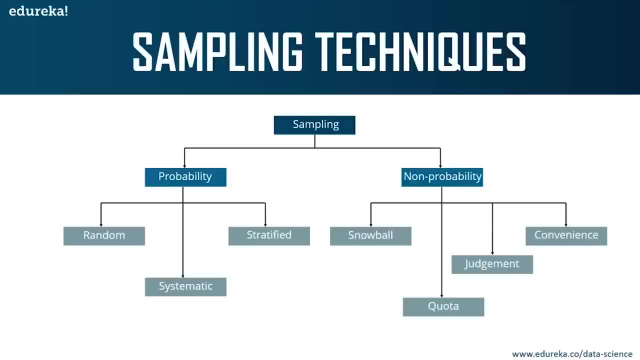 right now correct? Is it possible to survey each of these 42 million individuals about their health? Is it possible? Well, it might be possible, but this will take forever to do. Now, obviously it's not. it's not reasonable to go around knocking each door and asking for what does. 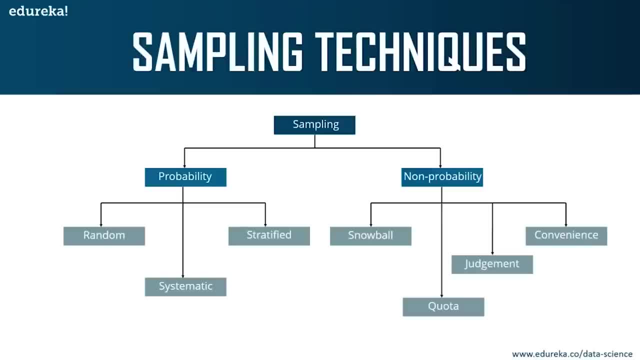 your teenage son eat and all of that, All right. This is not very reasonable. That's why sampling is used. It's a method wherein a sample of the population is studied in order to draw inference about the entire population, So it's basically a shortcut to studying the entire population. 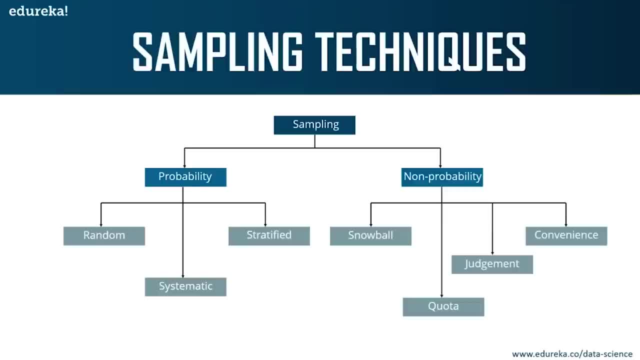 Instead of taking the entire population and finding out all the solutions, You're just going to take a part of the population that represents the entire population and you're going to perform all your statistical analysis, your inferential statistics, on that small sample. All right, 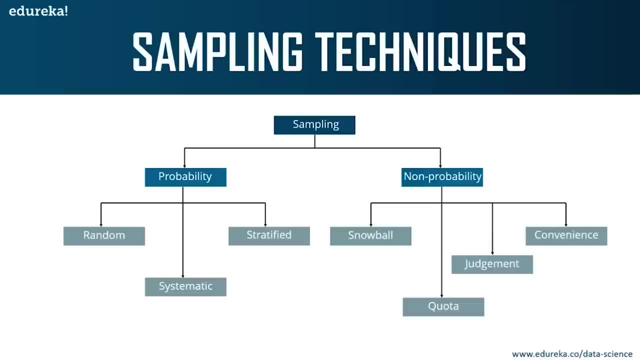 And that sample basically represents the entire population. All right, So I'm sure I've made this clear to all: what is sample and what is population. Now there are two main types of sampling techniques that I'll discuss today. We have probability sampling and non-probability sampling. 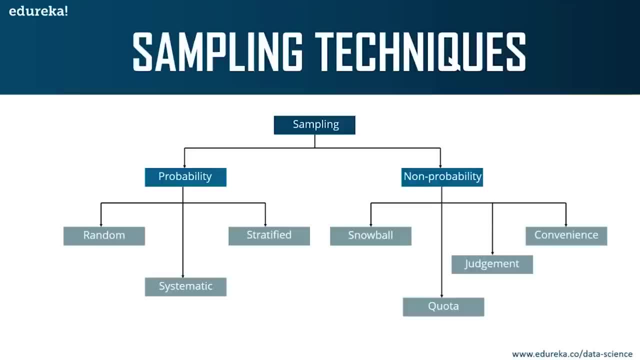 Now, in this video we'll only be focusing on probability sampling techniques, because non-probability sampling is not within the scope of this video. All right, we'll only discuss the probability. But because we're focusing on statistics and probability correct now again under probability sampling. 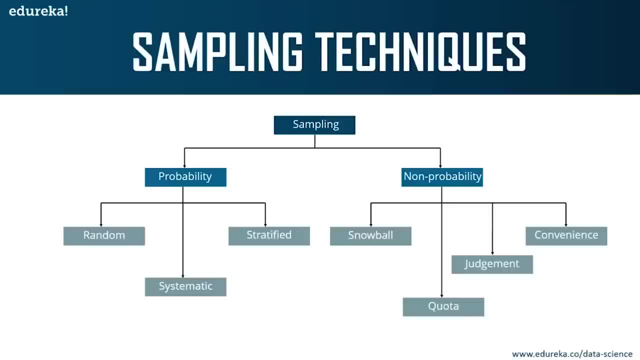 We have three different types. We have random sampling, systematic and stratified sampling- All right, and just to mention the different types of non-probability samplings, We have snowball, quota judgment and convenient sampling- All right. now, guys in this session, 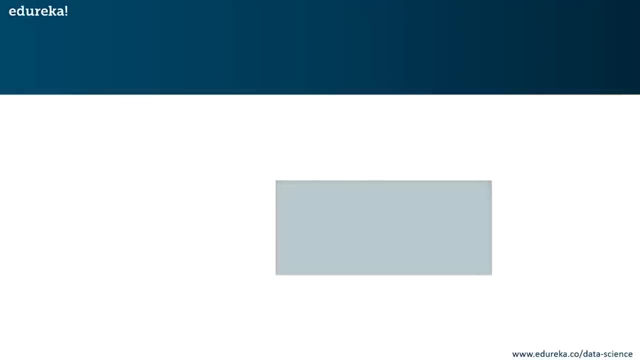 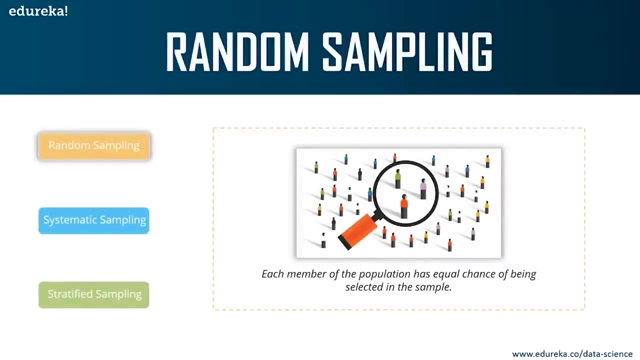 I'll only be focusing on probability, So let's move on and look at the different types of probability sampling. So what is probability sampling? It is a sampling technique in which samples from a large population are chosen by using the theory of probability. All right? 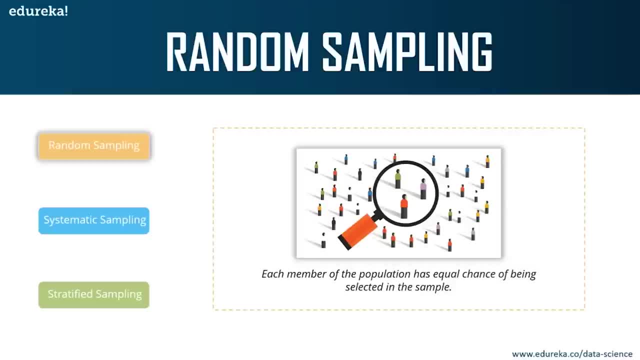 So there are three types of probability sampling. All right. First, we have the random sampling. Now, in this method, each member of the population has an equal chance of being selected in the sample. All right, So each and every individual or each and every object in the population. 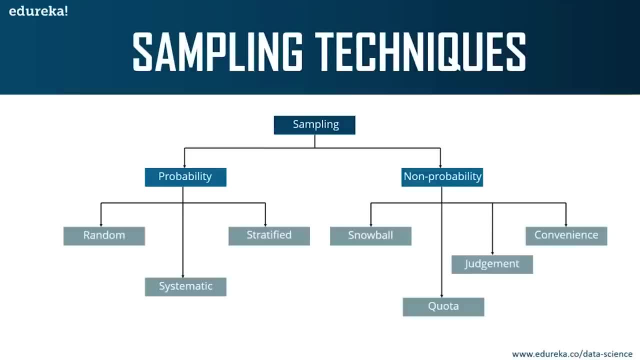 techniques, because non-probability sampling is not within the scope of this video. All right, we'll only discuss the probability part, because we're focusing on statistics and probability, correct. now again, under probability sampling, We have three different types. We have random sampling, systematic and stratified sampling. 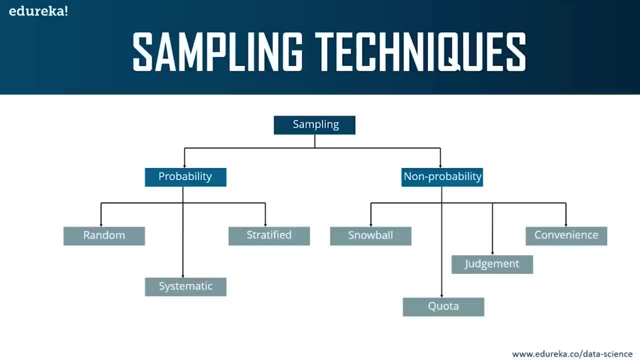 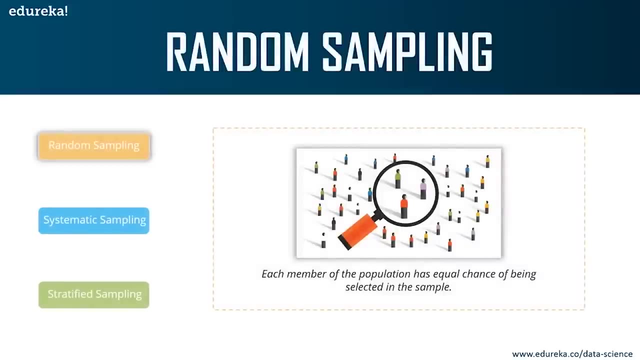 All right, and just to mention the different types of non-probability samplings, We have snowball quota judgment and convenient sampling. All right now, guys, in this session I'll only be focusing on probability, So let's move on and look at the different types of probability sampling. 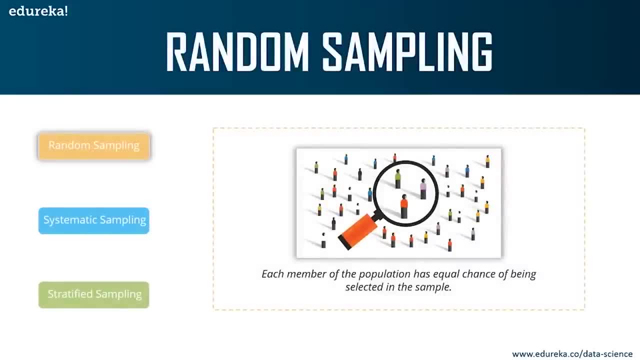 So what is probability sampling? It is a sampling Technique in which samples from a large population are chosen by using the theory of probability. All right, So there are three types of probability sampling, All right. First we have the random sampling. 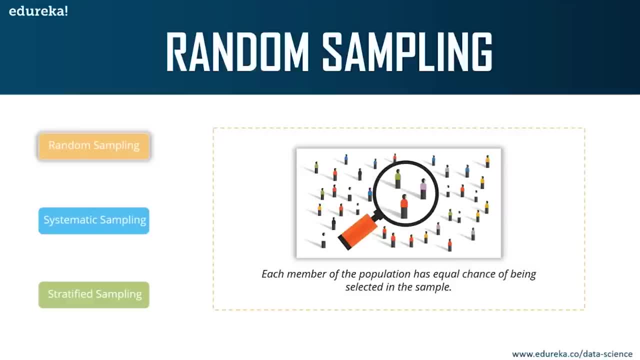 Now, in this method, each member of the population has an equal chance of being selected in the sample. All right, So each and every individual or each and every object in the population has an equal chance of being a part of the sample. That's what random sampling is. 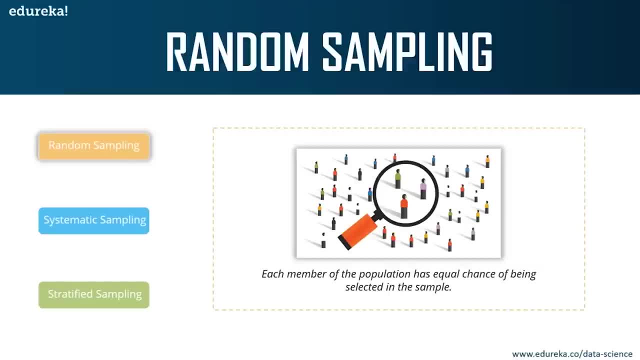 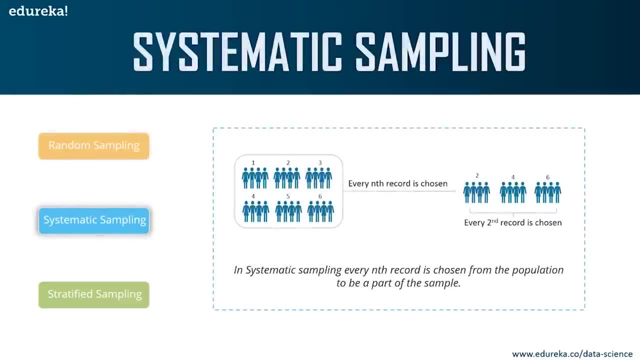 All about. okay, you're randomly going to select any individual or any object, So this way, each individual has an equal chance of being selected, Correct? Next we have systematic sampling. now, in systematic sampling, every nth record is chosen from the population to be a part of the sample. 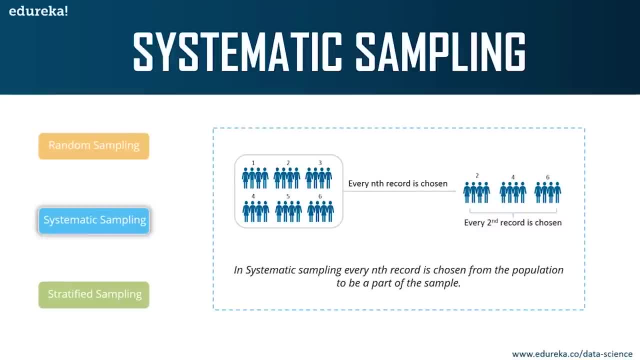 All, right, now refer this image that I've shown over here. out of these six groups, every second group is chosen as a sample. Okay, so every second record is chosen here, and this is how systematic sampling works. Okay, you're randomly selecting the nth record and you're going to add. 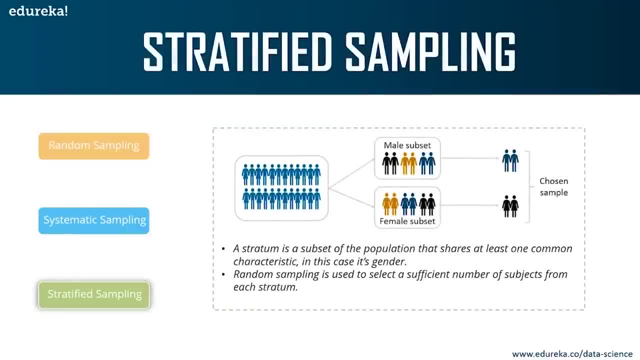 that to your sample. Next, we have stratified sampling now. in this type of technique, a stratum is used to form samples from a large population. So what is a stratum? a stratum is basically a subset of the population that shares at least one common characteristics. 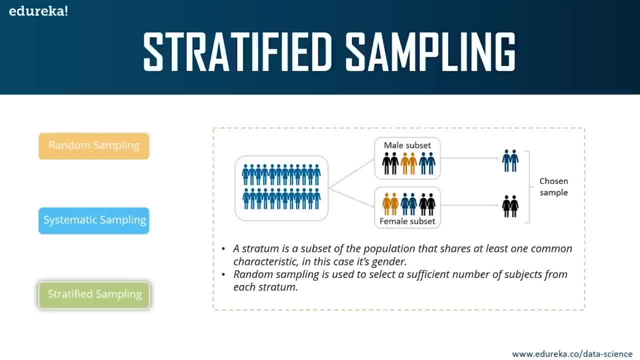 So let's say that your population has a, Both male and female, so you can create two stratums out of this. one will have only the male subset and the other will have the female subset. All right, This is what stratum is. It is basically a subset of the population that shares at least one common 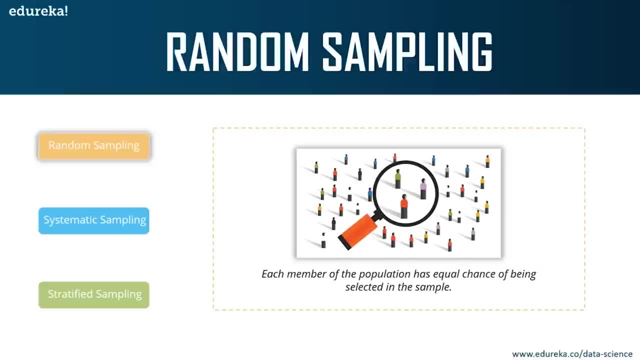 Has an equal chance of being a part of the sample. That's what random sampling is all about. Okay, you're randomly going to select any individual or any object, So this way, each individual has an equal chance of being selected, Correct? Next we have systematic sampling. 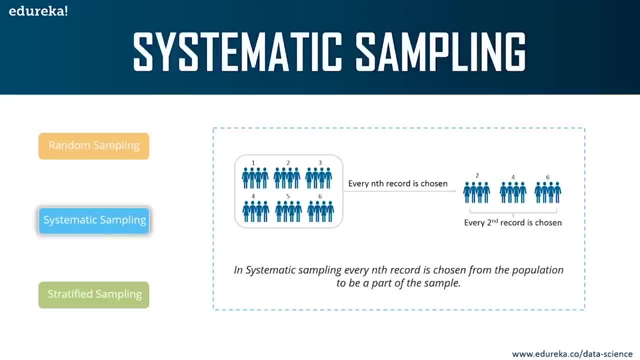 Now, in systematic sampling, every nth record is chosen from the population to be a part of the sample. All right, now refer this image that I've shown over here: Out of these six groups, every second group is chosen as a sample. Okay, so every second record is chosen here, and this is how systematic sampling works. 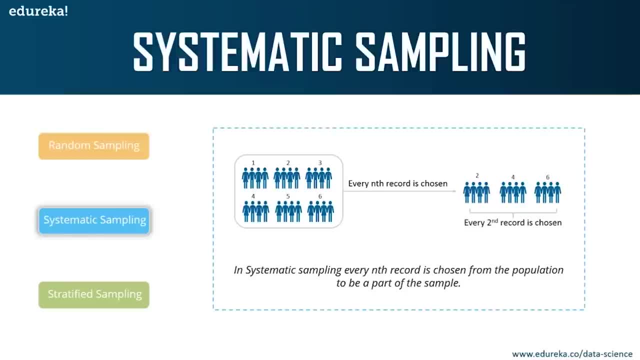 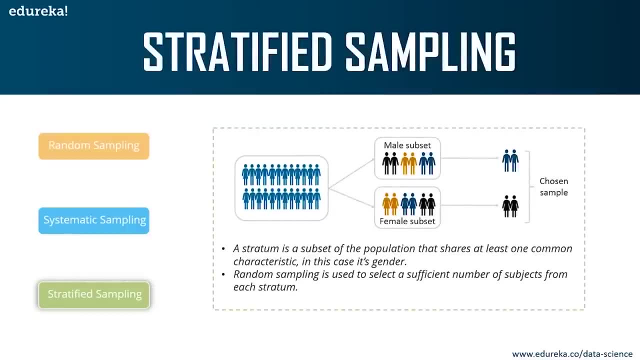 Okay, you're randomly selecting the nth record and you're going to add that to your sample. Next we have stratified sampling. Now, in this type of technique, a stratum is used to form samples from a large population. So what is a stratum? 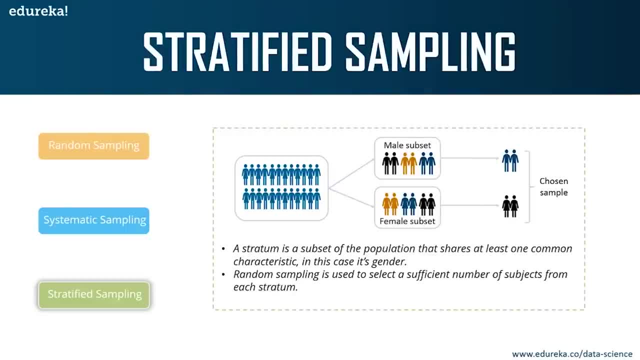 A stratum is basically a subset of the population That shares at least one common characteristics. So let's say that your population has a mix of both male and female. So you can create two stratums out of this. one will have only the male subset and the other will have the female subset. 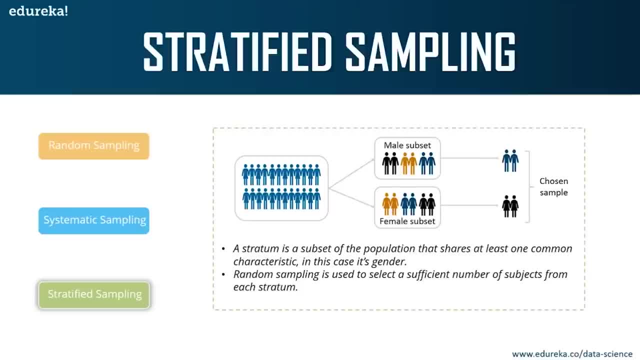 All right, This is what stratum is. It is basically a subset of the population that shares at least one common characteristics. All right, in our example, it is gender. So after you've created a stratum, you're going to use random sampling on these two. 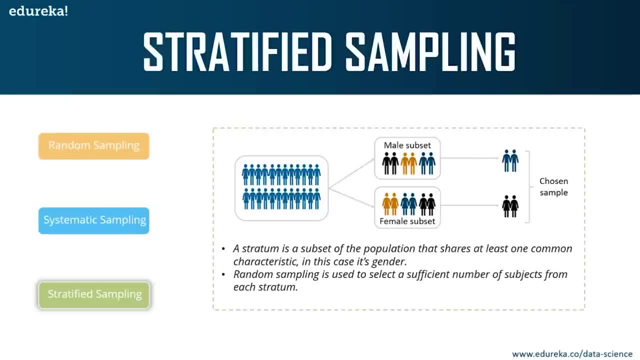 Stratums and you're going to choose a final sample, So random sampling, meaning that all of the individuals in each of the stratum will have an equal chance of being selected in the sample, Correct? So, guys, these were the three different types of sampling techniques. 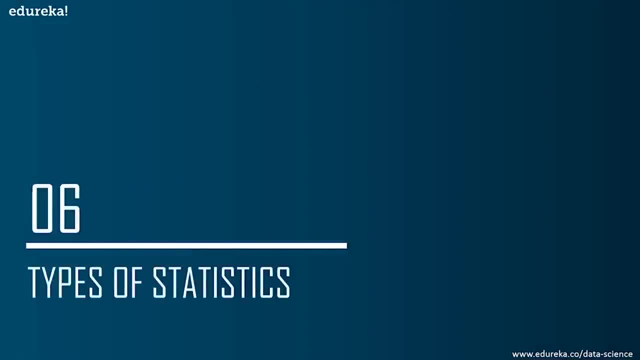 Now let's move on and look at our next topic, which is the different types of statistics. So after this, we'll be looking at the more advanced concepts of statistics. All right, So far we discussed the basics of statistics, which is basic. 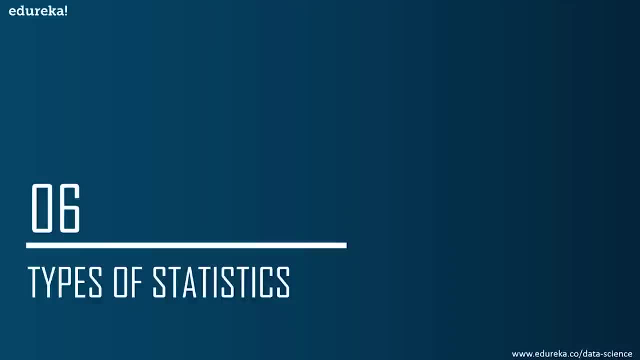 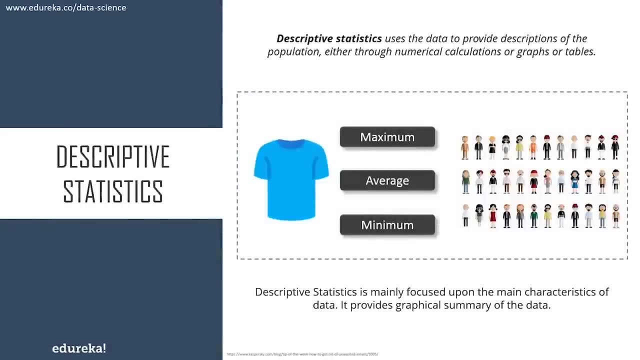 Basically, what is statistics? the different sampling techniques and the terminologies and statistics. All right, Now we look at the different types of statistics. So there are two major types of statistics: descriptive statistics and inferential statistics. in today's session, We'll be discussing both of these types of statistics in depth. 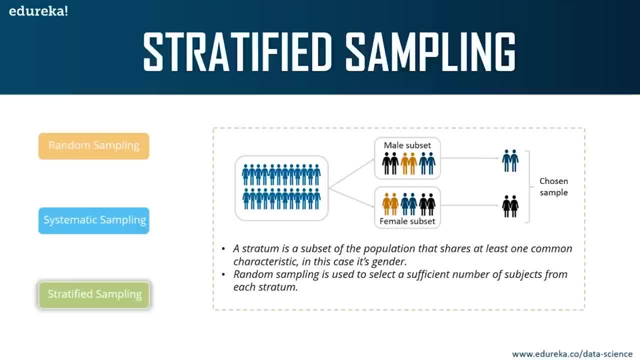 characteristics. All right, in our example it is gender. So, after you've created a stratum, you're going to use random sampling on these stratums and you're going to choose a final sample. So random sampling meaning that all of the Individuals in each of the stratum will have an equal chance of being. 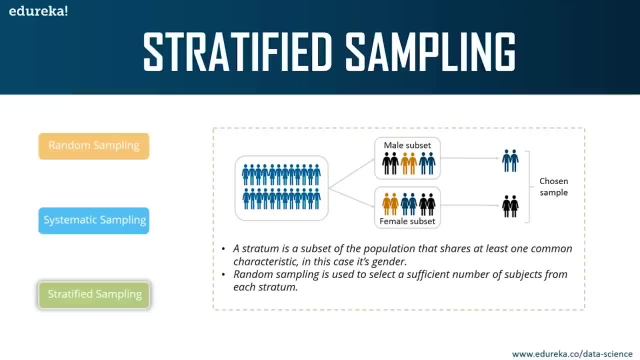 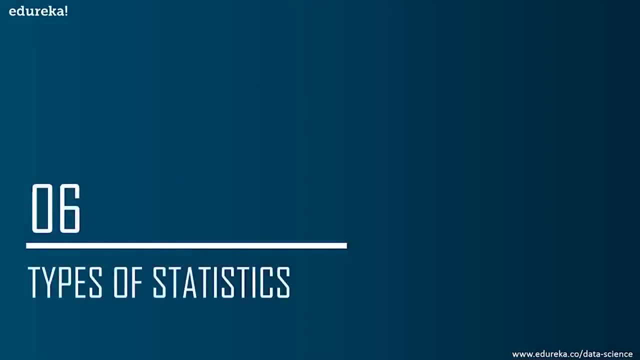 selected and the sample correct. So, guys, these were the three different types of sampling techniques. Now let's move on and look at our next topic, which is the different types of statistics. So after this will be looking at the more advanced concepts of statistics. 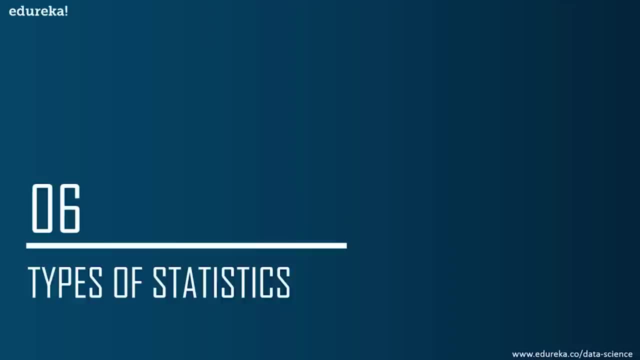 All right, So far we discussed the basics of statistics, which is basically what is statistics, the different sampling techniques and the terminologies and statistics. All right, Now we look at the different types of statistics. So there are two major types of statistics: descriptive statistics and 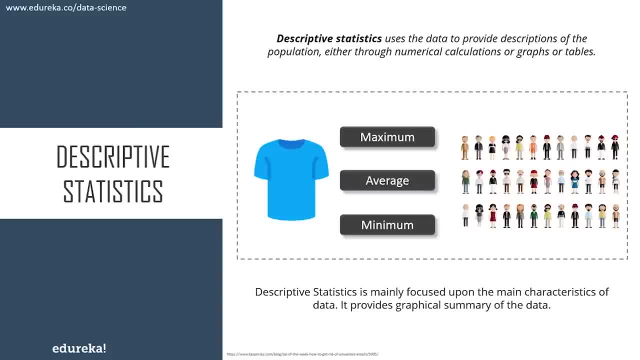 inferential statistics. in today's session, We'll be discussing both of these types of statistics in depth. right We'll also be looking at a demo which I'll be running in the R language in order to make you understand what exactly descriptive and inferential. 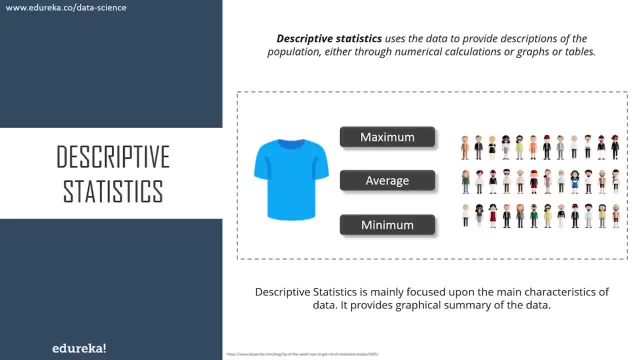 statistics is. So, guys, we're just going to look at the basics, So don't worry if you don't have much knowledge. I'm explaining everything from the basic level, All right. So, guys, descriptive statistics is a method which is used to describe and. 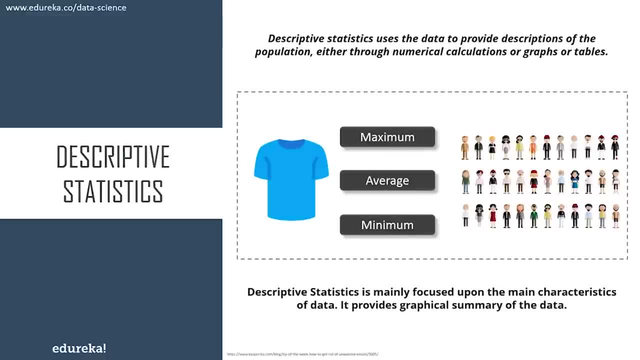 understand the features of specific data set by giving a short summary of the data. Okay, so it is mainly focused upon the characteristics of data. It also provides a graphical summary of the data. Now, in order to make you understand what descriptive statistics is, let's 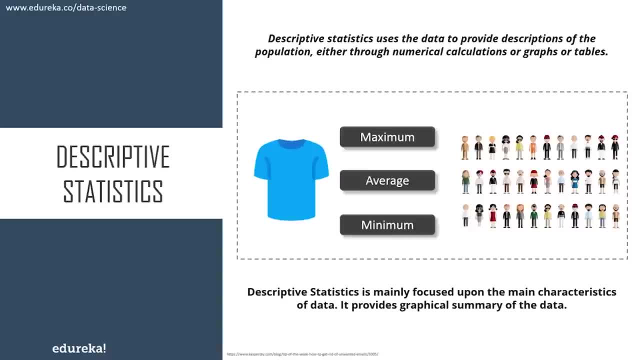 suppose that you want to gift all your classmates A t-shirt, so to study the average shirt size of a student in a classroom. So if you were to use descriptive statistics to study the average shirt size of students in your classroom, then what you would do is you would. 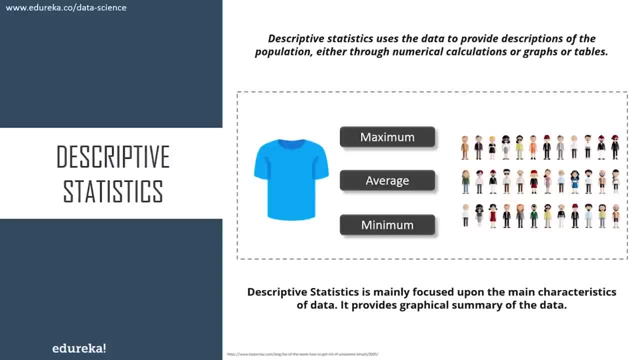 record the shirt size of all students in the class and then you would find out the maximum, minimum and average shirt size of the club. Okay, so coming to inferential statistics. inferential statistics makes inferences and predictions About a population based on the sample of data taken from the population. 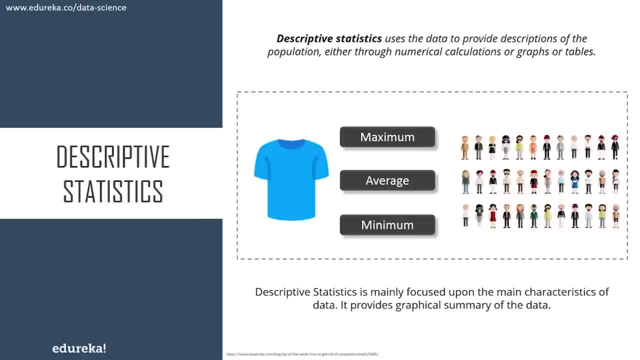 All right, We'll also be looking at a demo, which I'll be running in the our language, in order to make you understand what exactly descriptive and inferential statistics are. So, guys, we're just going to look at the basics, So don't worry if you don't have much knowledge. 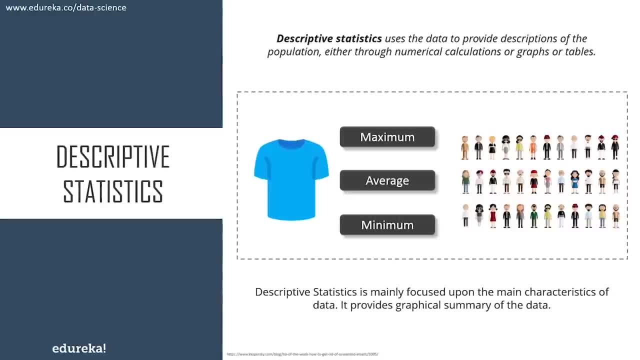 I'm explaining everything from the basic level, All right. So, guys, descriptive statistics is a method which is used to describe and understand the features of specific data set by giving a short summary of the data. Okay, so it is mainly focused upon the characteristics of data. 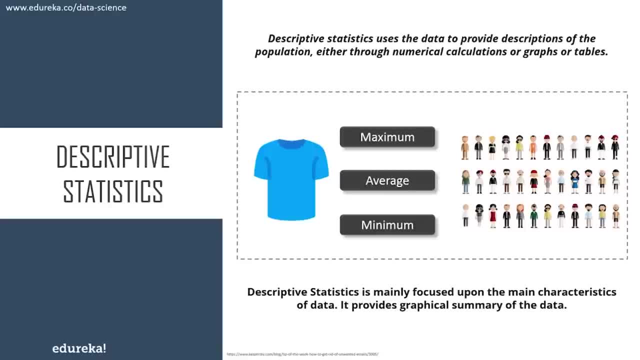 It also provides a graphical summary of the data. now, in order to make you understand, Descriptive statistics is: let's suppose that you want to gift all your classmates a t-shirt, So to study the average shirt size of a student in a classroom. So if you were to use descriptive statistics to study the average shirt size of students in your classroom, then what you would do is you would record the shirt. 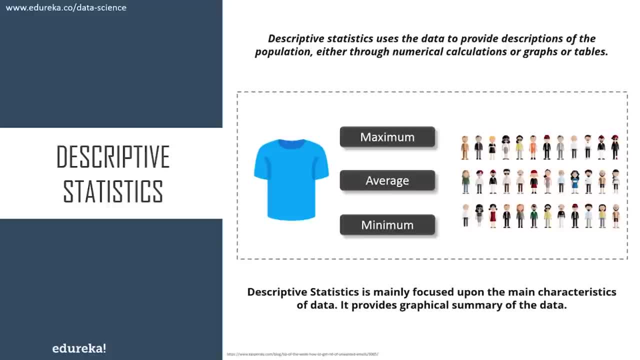 size of all students in the class and then you would find out the maximum, minimum and average shirt size of the club. Okay, so, coming to inferential statistics. Inferential statistics makes inferences and predictions about a population based on the sample of data taken from the population. 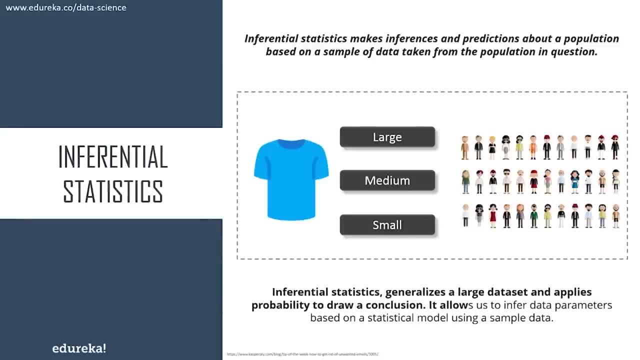 Okay so, in simple words, it generalizes a large data set and it applies probability to draw a conclusion. Okay so it allows you to infer data parameters based on a statistical model by using sample data. So if we consider the same example of finding the average shirt size of students in a class, 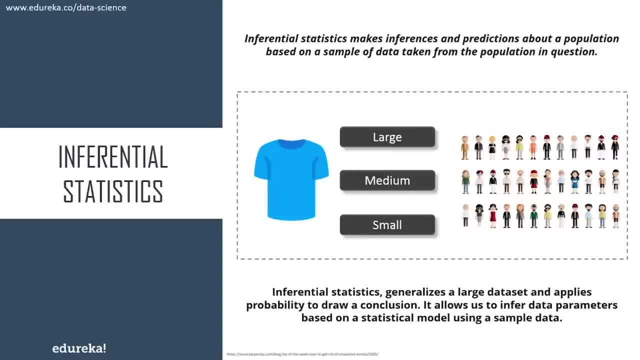 In inferential statistics you will take a sample set of the class, which is basically a few people from the entire class. All right, you already have had grouped the class into large, medium and small. All right. in this method, you basically build a statistical model and expand it for the entire population in the class. 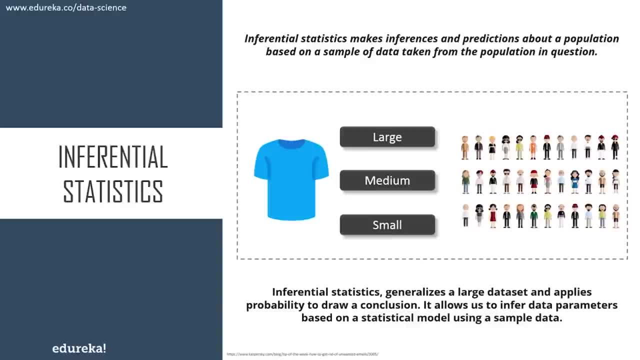 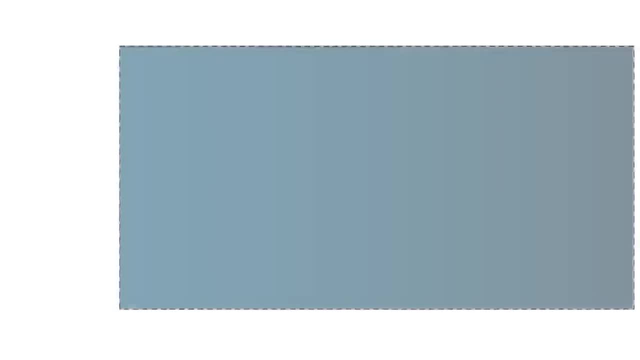 So, guys, there was a brief understanding of descriptive and inferential statistics. So that's the difference between descriptive and inferential. Now, in the next section, we'll go in-depth about description, Descriptive statistics. All right, so let's discuss more about descriptive statistics. 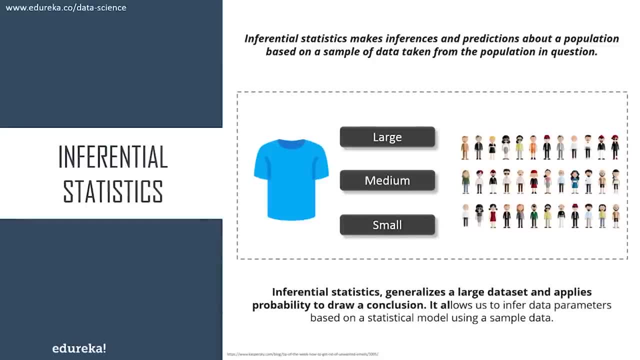 Okay so, in simple words, it generalizes a large data set and it applies probability to draw a conclusion. Okay so it allows you to infer data parameters based on a statistical model by using sample data. So if we consider the same example of finding the average shirt size of 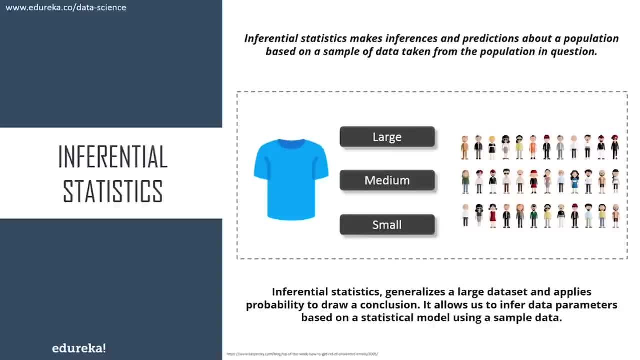 students in a class. in inferential statistics you will take a sample set of the class, Which is Basically a few people from the entire class. All right, you already have had grouped the class into large, medium and small. All right, in this method. 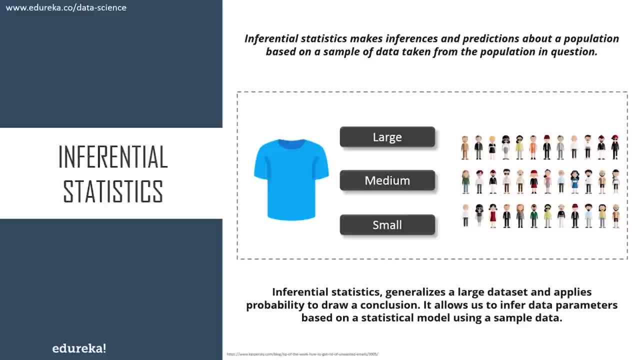 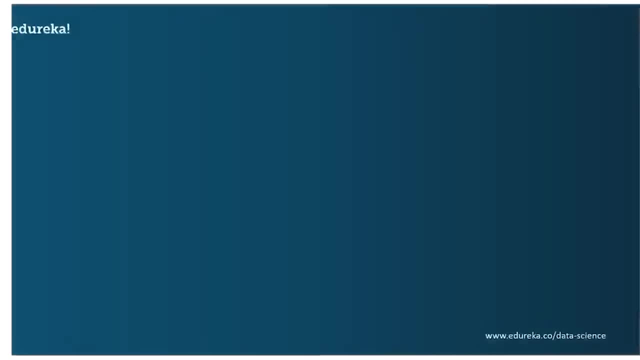 You basically build a statistical model and expand it for the entire population in the class. So, guys, there was a brief understanding of descriptive and inferential statistics. So that's the difference between descriptive and inferential. Now, in the next section, we'll go in depth about descriptive statistics. 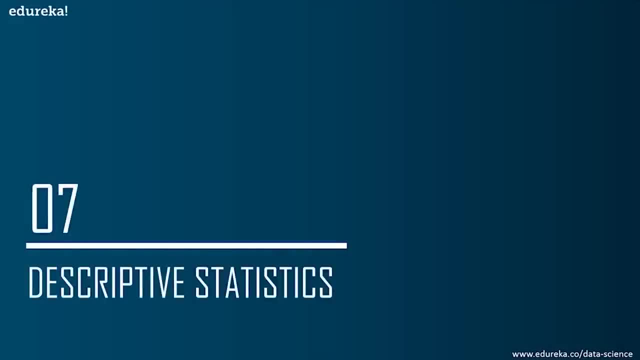 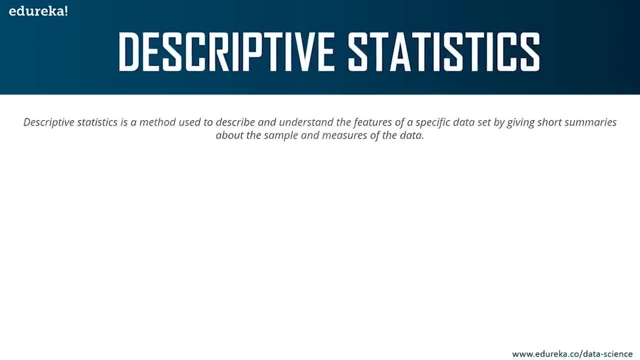 All right, so let's discuss more About descriptive statistics. So, like I mentioned earlier, descriptive statistics is a method that is used to describe and understand the features of a specific data set by giving short summaries about the sample and measures of the data. There are two important measures in descriptive statistics. 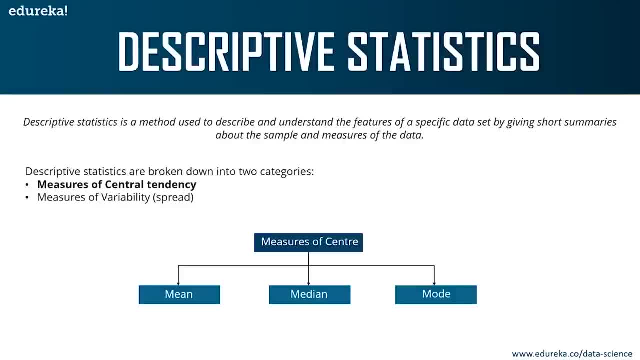 We have measure of central tendency, which is also known as measure of center, and we have measures of variability- This is also known as measures of spread. So measures Of center include mean, median and mode. Now, what is measures of center? measures of the center are statistical. 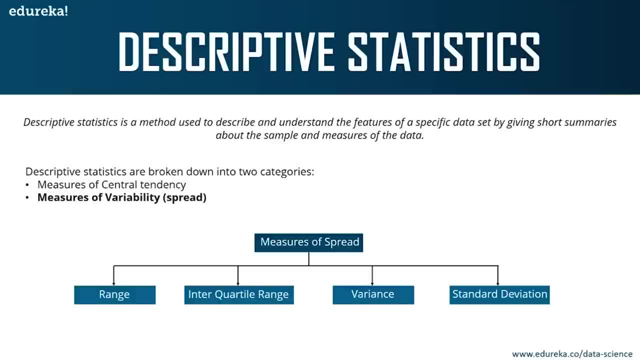 measures that represent the summary of a data set. Okay, the three main measures of center are mean, median and mode. coming to measures of variability or measures of spread, We have range, interquartile range, variance and standard deviation. All right, So now let's discuss each of these measures in a little more depth. 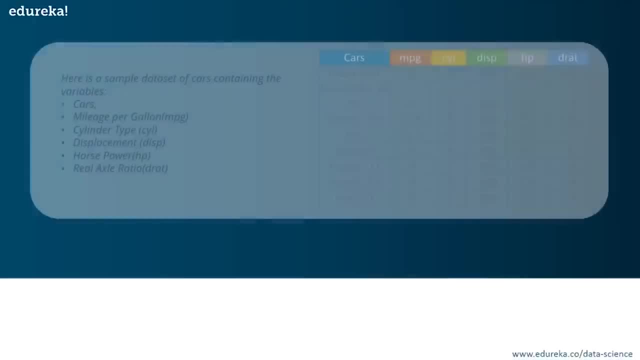 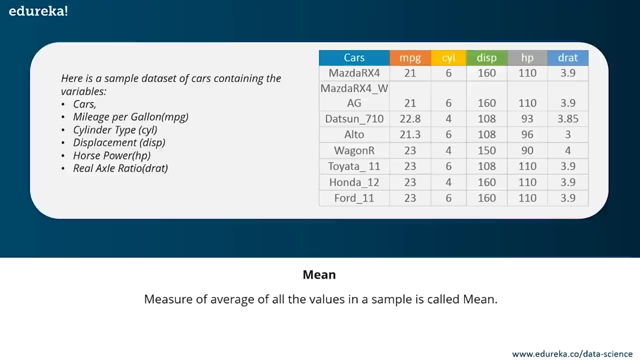 Starting with the measures of center. I'm sure all of you know what the mean is. mean is basically the measure of the average of all the values in a sample. Okay, so it's basically the average of all the values in a sample. How do you measure the mean? 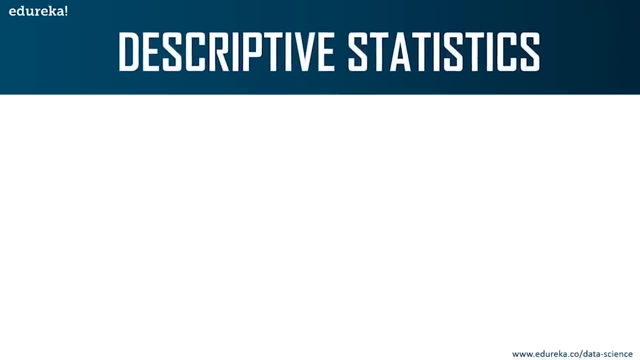 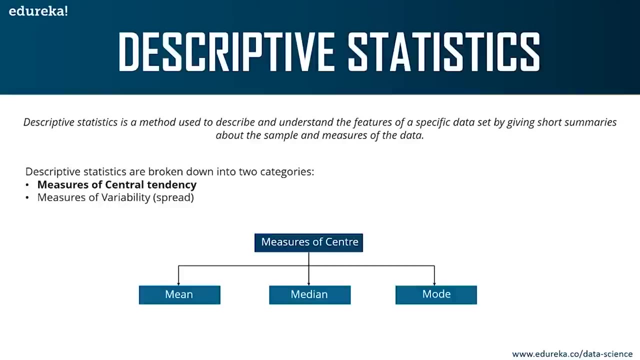 So, like I mentioned earlier, descriptive statistics is a method that is used to describe and understand the features of a specific data set by giving short summaries about the sample and measures of the data. There are two important measures in descriptive statistics: We have measure of central tendency, which is also known as measure of center, and we have measures of variability. 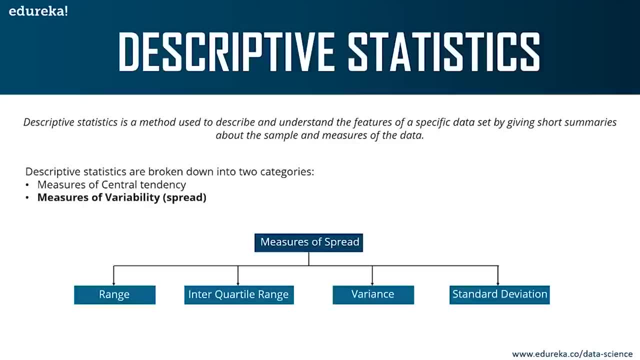 This is also known as measures of spread. So measures of center include mean, median and mode. Now, what is measures of center? Measures of the center are statistical measures that represent the summary of a data set. Okay, the three main measures of center are mean, median and mode. 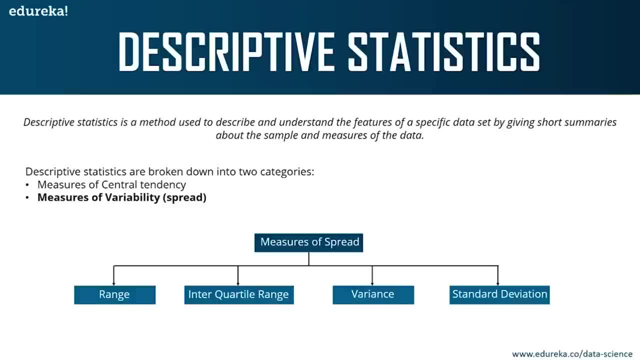 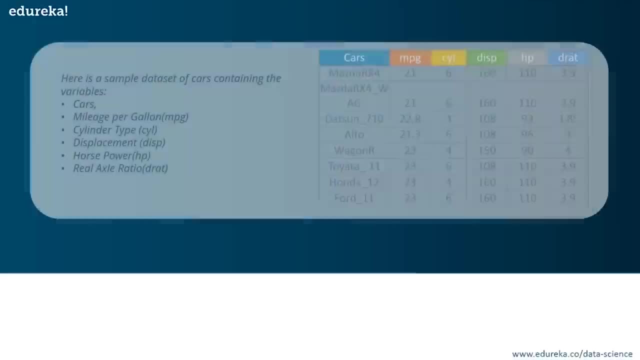 Coming to measures of variability or measures of spread. we have range, interquartile range variance and standard deviation. All right, So now let's discuss each of these measures in a little more depth, starting with the measures of center. I'm sure all of you know what the mean is. 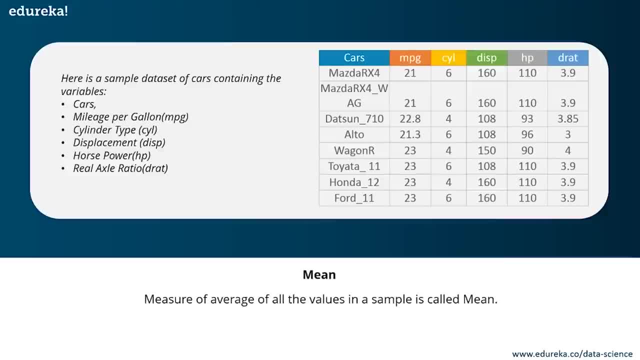 Mean is basically the measure of the average of all the values in a sample. Okay, so it's basically the average of all the values in a sample. How do you measure the mean? I hope all of you know how the mean is measured. 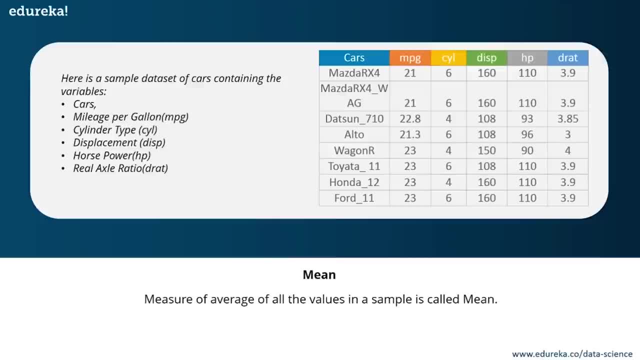 If there are 10 numbers and you want to find the mean of these 10 numbers, all you have to do is you have to add up all the 10 numbers and you have to divide it by 10.. 10 here represents the number of samples in your data set. 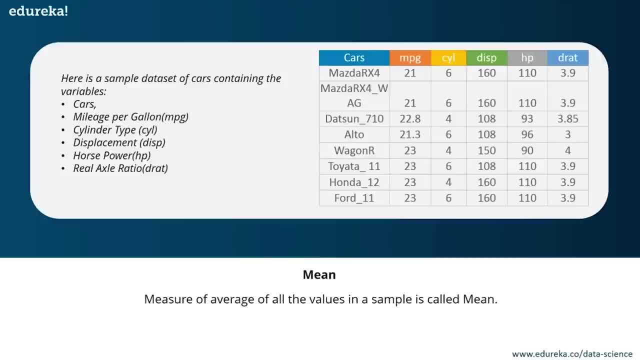 All right, since we have 10 numbers, we're going to divide this by 10.. All right, this will give us the average or the mean. So to better understand the measures of central tendency, let's look at an example Now. 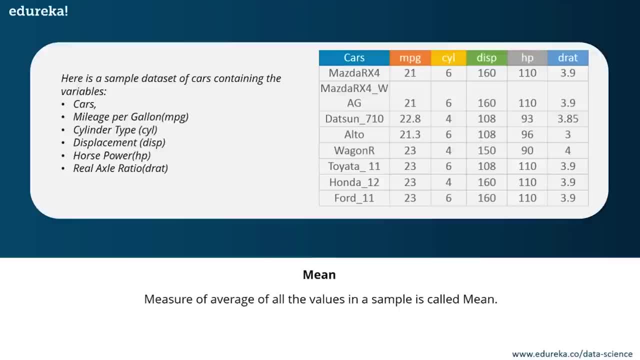 the data set over here is basically the cars data set and it contains a few variables. All right, it has something known as cars. It has mileage per gallon cylinder type displacement. It has mileage per gallon cylinder type displacement, horsepower and real axle ratio. 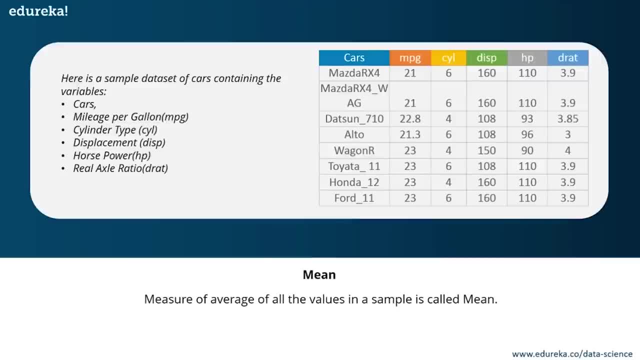 All right, all of these measures are related to cars, Okay, So what you're going to do is you're going to use descriptive analysis and you're going to analyze each of the variables in the sample data set for the mean standard deviation median. 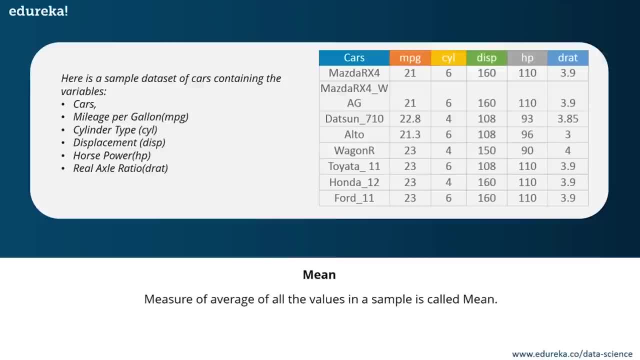 I hope all of you know how the mean is measured. If there are 10 numbers and you want to find the mean of these 10 numbers, All you have to do is you have to add up all the 10 numbers and you have to divide it by 10. 10 your represents the number. 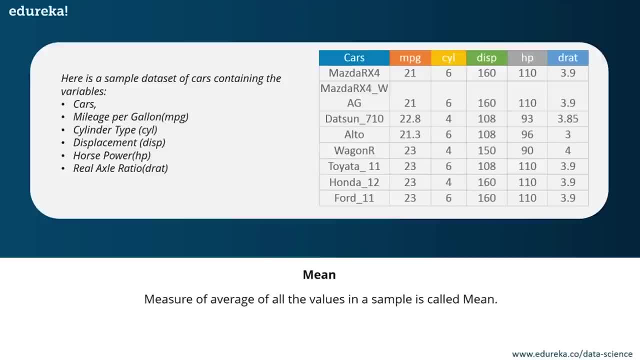 Of samples in your data set. All right, since we have 10 numbers, we're going to divide this by 10.. All right, this will give us the average or the mean. So, to better understand the measures of central tendency, Let's look at an example. 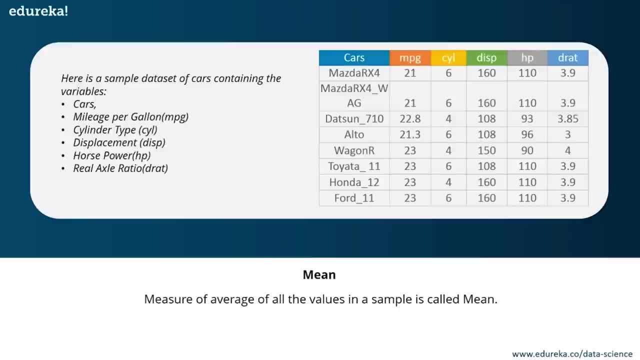 Now, the data set over here is basically the cars data set, and it contains a few variables. All right, It has something known as cars. It has mileage per gallon, cylinder type, displacement, horsepower and real axle ratio. All right, All of these measures are related to cars. 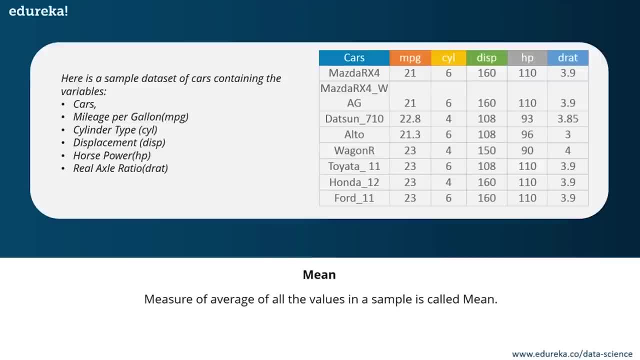 Okay. So what you're going to do is you're going to use descriptive analysis and you're going to analyze each of the variables in the sample data set for the mean, standard, deviation, median, more and so on. So let's say that you want to find out the mean or the average horsepower. 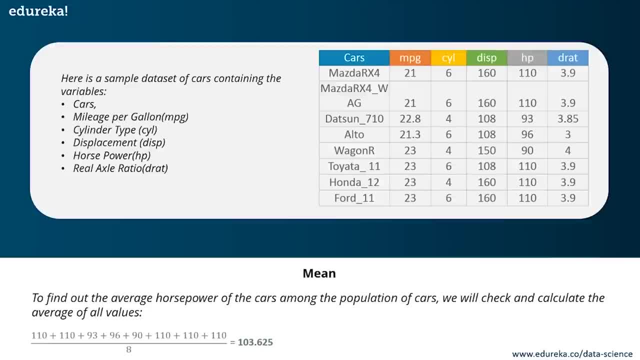 of the cars among the population of cars. Like I mentioned earlier, what you do is you will check the average of all the values. So in this case we'll take the sum of the horsepower Of each car and we'll divide that by the total number of cars. 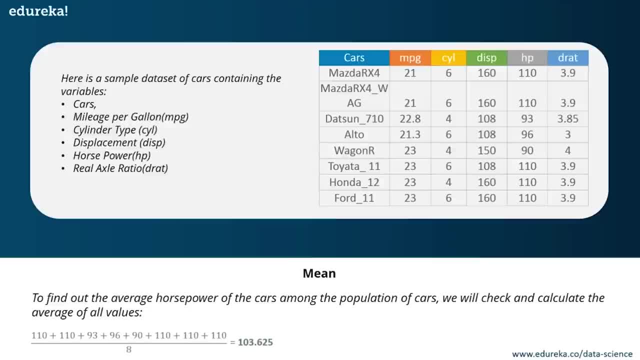 Okay, That's exactly what I've done here in the calculation part. So this 110 basically represents the horsepower for the first car, All right. Similarly, I've just added up all the values of horsepower for each of the cars and I've divided it by 8. now, 8 is basically the number of cars in our data set. 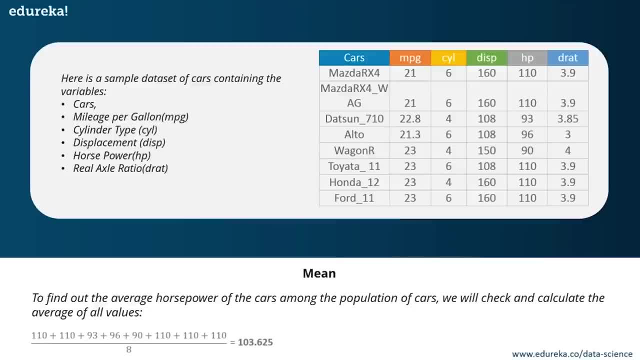 All right. So 103.625 is what our mean is, Or the average of horsepower is all right. Now let's understand what median is with an example. Okay, so to define median: median is basically a measure of the central value of the sample set is called the median. 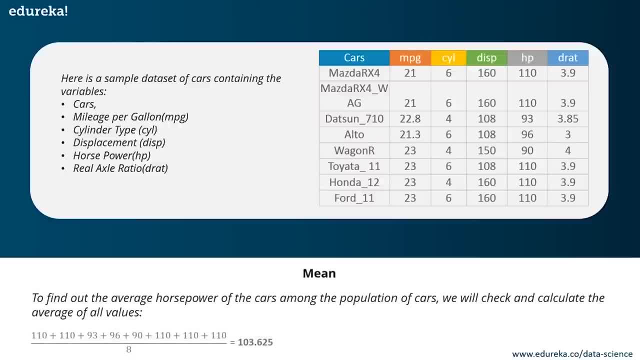 more and so on. So let's say that you want to find out the mean or the average horsepower of the cars among the population of cars. Like I mentioned earlier, what you do is you will check the average of all The values. So in this case, 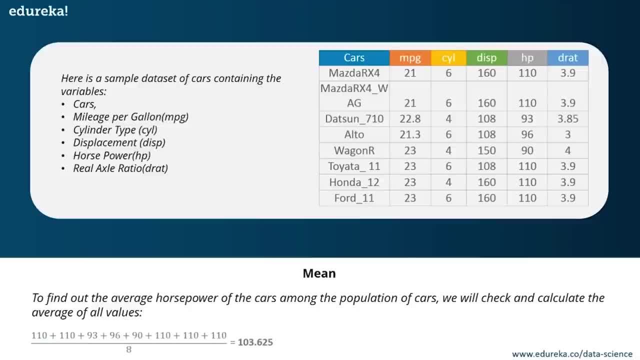 we'll take the sum of the horsepower of each car and we'll divide that by the total number of cars. Okay, that's exactly what I've done here in the calculation part. So this 110 basically represents the horsepower for the first car. 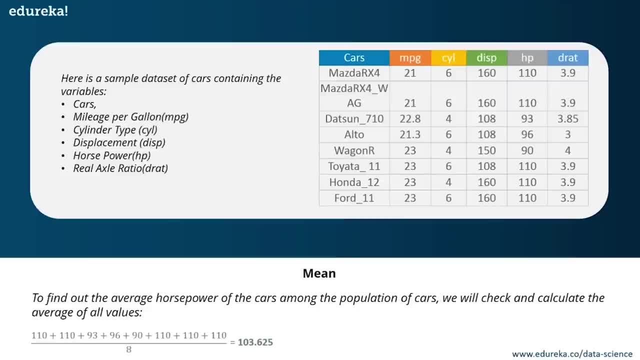 All right. Similarly, I've just added up all the values of horsepower for each of the cars and I've divided it by eight. Now, eight is basically the number of cars in our data set. All right, So 103.625 is what our mean is, or the average of horsepower is. 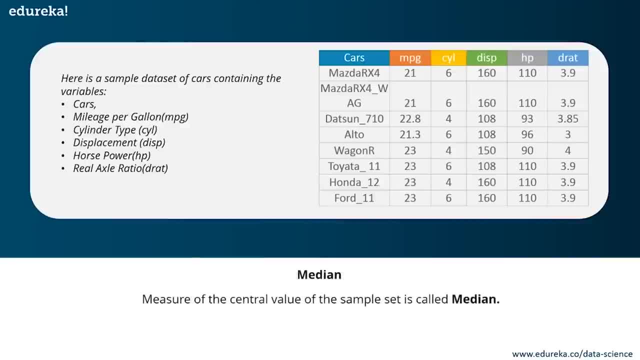 All right, Now let's understand what median is with an example. Okay, So to define median, median is basically a measure of the central value of the sample set is called the median. All right, you can see that it is a middle value. 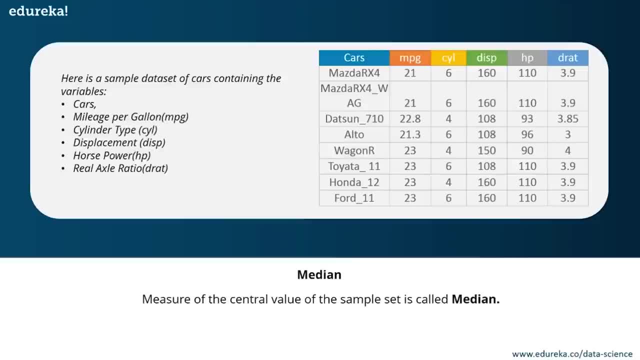 So if you want to find out the center value of the mileage per gallon among the population of cars first, what we'll do is we'll Range the mpg values in ascending or descending order and choose a middle value. All right in this case. 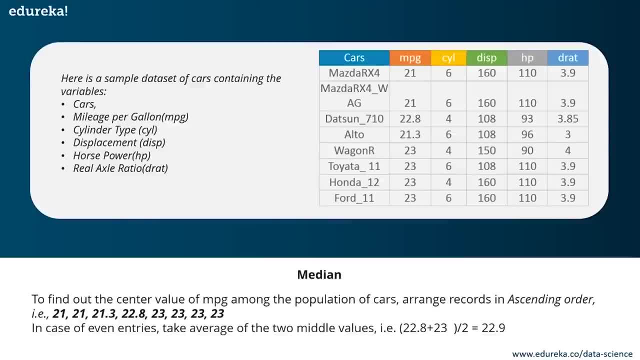 since we have eight values. right, we have eight values, which is an even entry. So whenever you have even number of data points or samples in your data set, then you're going to take the average of the two middle values. If we had nine values over here, 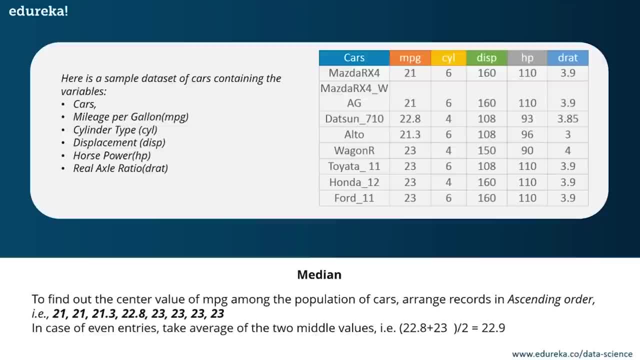 we can easily figure out the middle value and, you know, choose that as a median. But since they're even number of values, we're going to take the average of the two middle values. All right, So 22.8 and 23 are my two middle values and I'm taking the mean of those two and hence I get 22.9,. 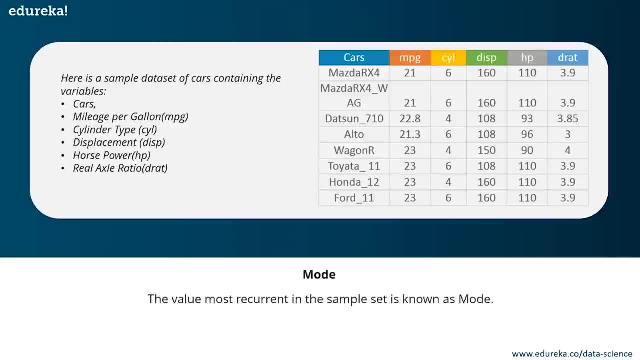 which is my median. All right, Lastly, let's look at how mode is calculated. So what is mode? and the value that is most recurrent in the sample set is known as mode, or basically the value that occurs most often. Okay, that is known as mode. 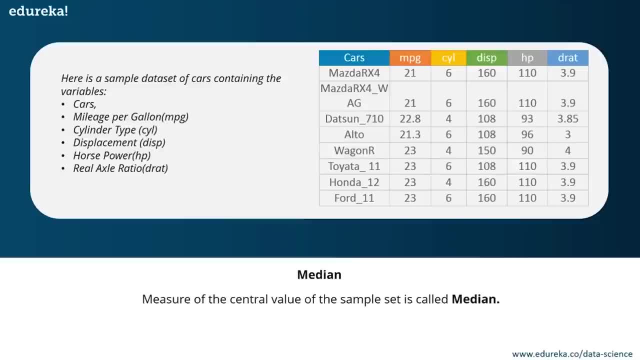 All right, you can see that it is a middle value. So if you want to find out the center value of the mileage per gallon among the population of cars first, what we'll do is we'll arrange the mpg values in ascending or descending order. 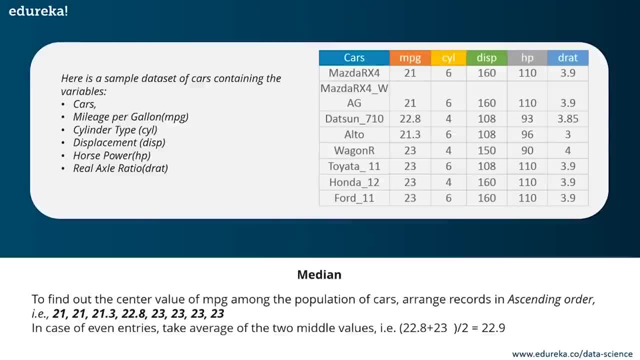 And choose a middle value. All right in this case, since we have eight values. right, We have eight values, which is an even entry. So whenever you have even number of data points or samples in your data set, then you're going to take the average of the two middle values. 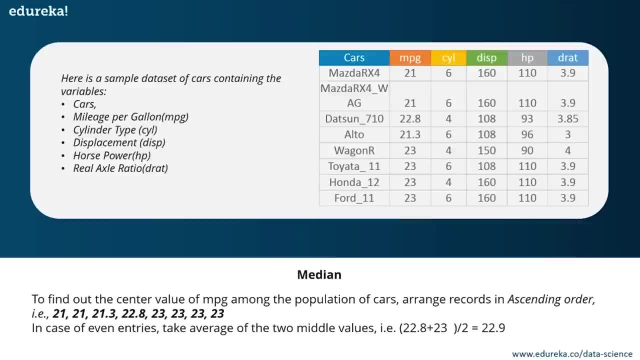 If we had nine values over here, we can easily figure out the middle value and, you know, choose that as a median. But since there are even number of values, we're going to take the average of the two middle values, All right. 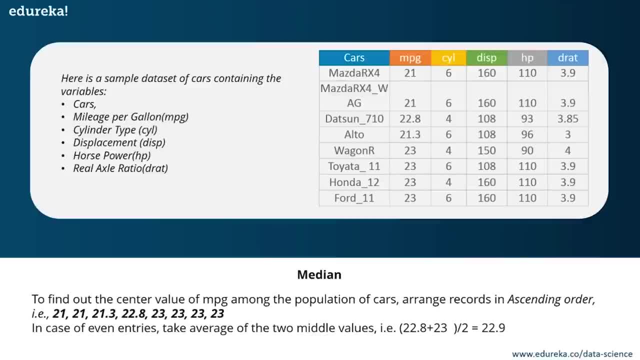 So 22.8 and 23 are my two middle values and I'm taking the mean of those two and hence I get 22.9, which is my median. All right, Lastly, let's look at how mode is calculated. So what is mode and the value that is most recurrent in the sample set. 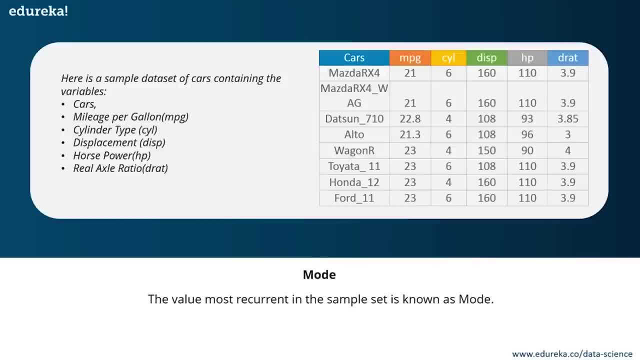 is known as mode, or basically the value that occurs most often. Okay, that is known as mode. So let's say that we want to find out the most common type of cylinder among the population of cars. All we have to do is we will check the value which is repeated: the. 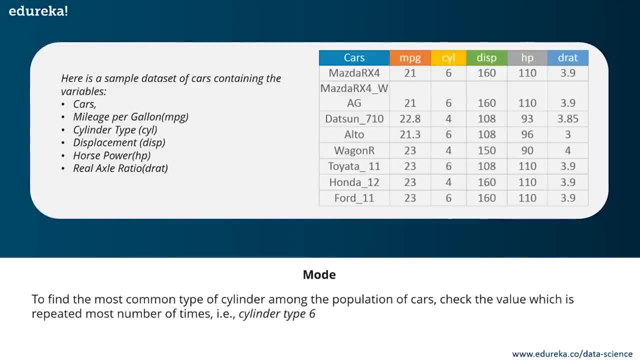 most number of times. here We can see that the cylinders come in two types. We have cylinder of type 4 and cylinder of type 6, right. So take a look at the data set. You can see that the most recurring value is 6, right. 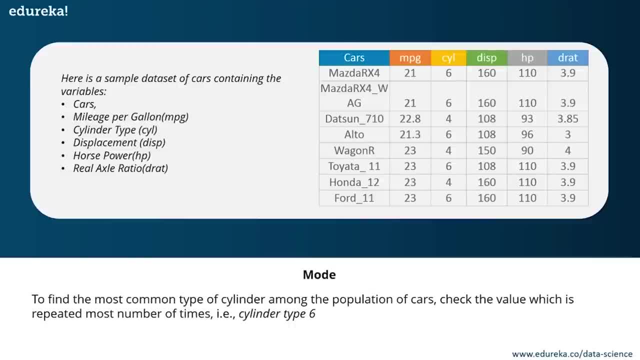 We have 1, 2, 3, 4 and 5, we have 5, 6 and we have 1, 2, 3.. Yeah, we have 3, 4 type cylinders and 5. 6 type cylinders. So basically, we have 3, 4 type cylinders and we have 5, 6 type cylinders. 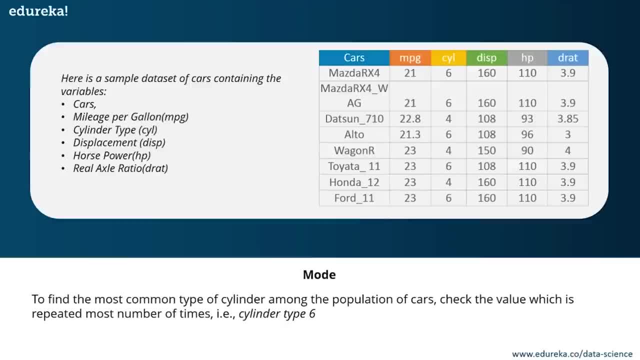 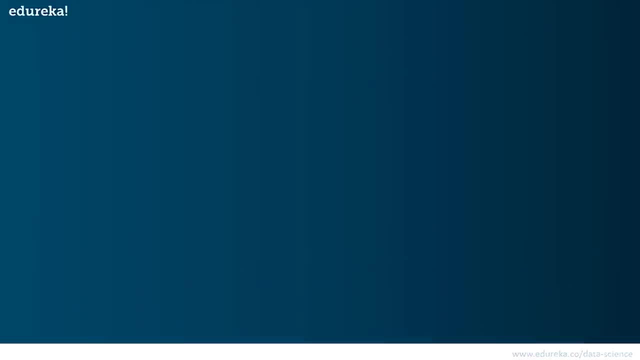 All right, So our mode is going to be 6, since 6 is more recurrent than 4.. So, guys, those were the measures of the center, or the measures of central tendency. Now let's move on and look at the measures of the spread. 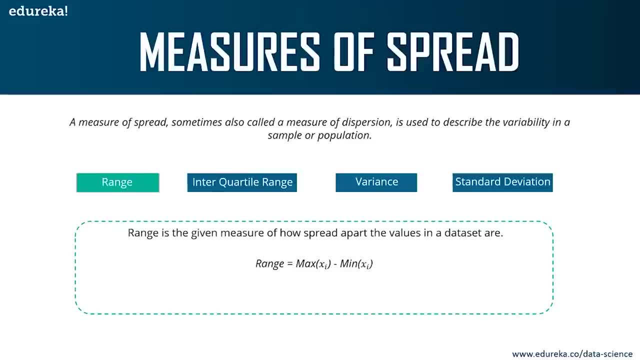 All right, Now, what is the measure of spread? a measure of spread, sometimes also called as measure of dispersion, is used to describe the variability in a sample or population. Okay, you can think of it as some sort of deviation in the sample, All right. 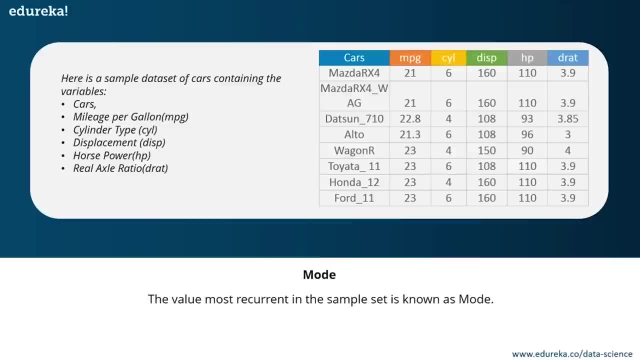 So let's say that we want to find out the most The most common type of cylinder among the population of cars. What we have to do is we will check the value which is repeated the most number of times. here We can see that the cylinders come in two types. 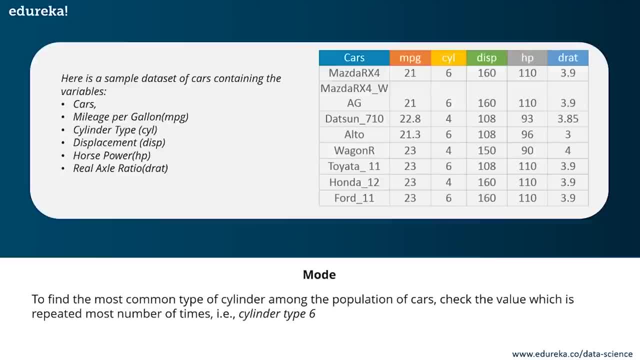 We have cylinder of type 4 and cylinder of type 6, right? So take a look at the data set. You can see that the most recurring value is 6, right. We have 1, 2, 3, 4 and 5. we have 5, 6 and we have 1, 2, 3.. 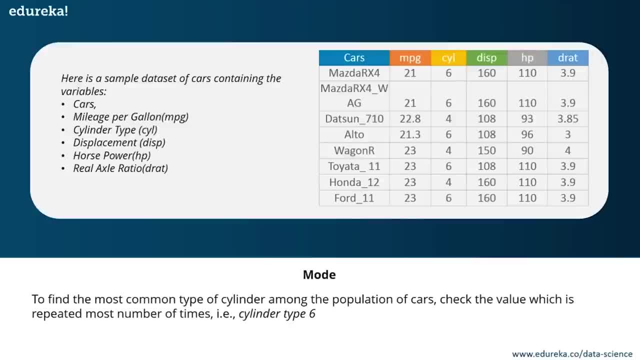 Yeah, we have 3- 4 type cylinders and 5- 6 type cylinders. So basically, we have 3- 4 type cylinders and we have 5- 6 type cylinders. All right, So our mode is going to be 6, since 6 is more recurrent than 4.. 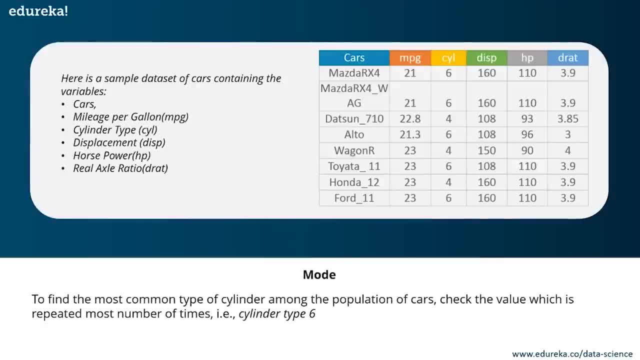 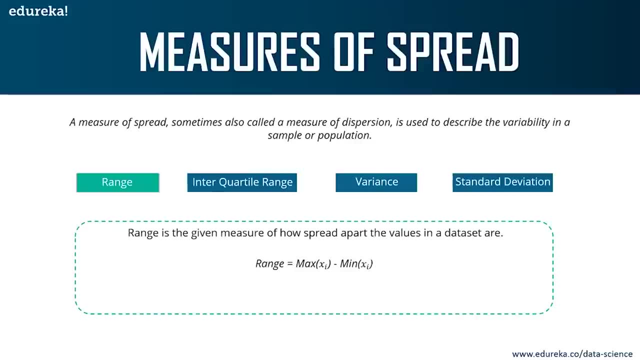 So, guys, those were the measures of the center, or the measures of central tendency. Now let's move on and look at the measures of the spread. All right, Now, what is the measure of spread? a measure of spread, Sometimes also called as measure of dispersion, is used to describe the variability in a sample or population. 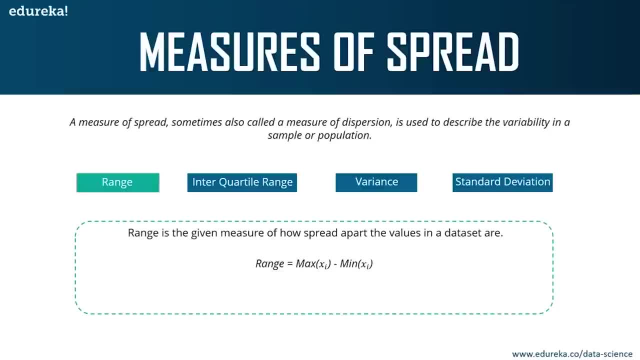 Okay, you can think of it as some sort of deviation in the sample. All right, so you measure this with the help of the different measure of spreads. We have range, interquartile range, variance and standard deviation. Now, range is pretty self-explanatory, right. 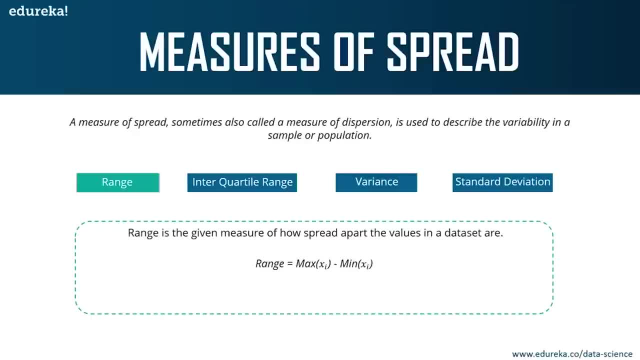 It is the given measure of how, spread apart, the values in a data set are. the range can be calculated as shown in this formula. So you basically going to subtract the maximum value in your data set from the minimum value in your data set. That's how you calculate the range of the data. 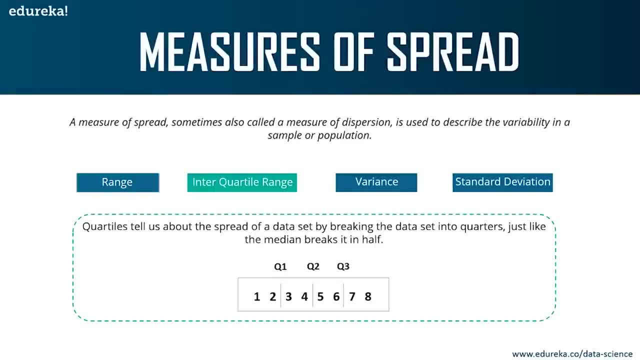 All right. Next we have interquartile range. So before we discuss interquartile range, let's understand what a quartile is. All right. So quarter is basically tell us about the spread of a data set by breaking the data set into different quarters. 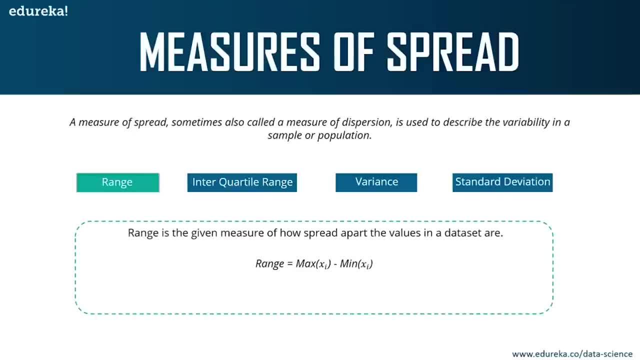 So you measure this with the help of the different measure of spreads. We have range, interquartile range, variance and standard deviation. Now, range is pretty self-explanatory, right. It is the given measure of how spread apart the values in a data set. 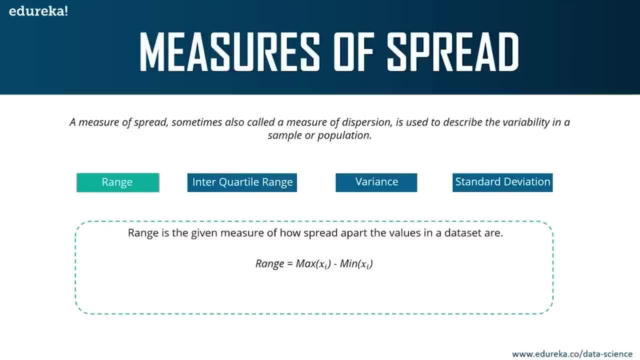 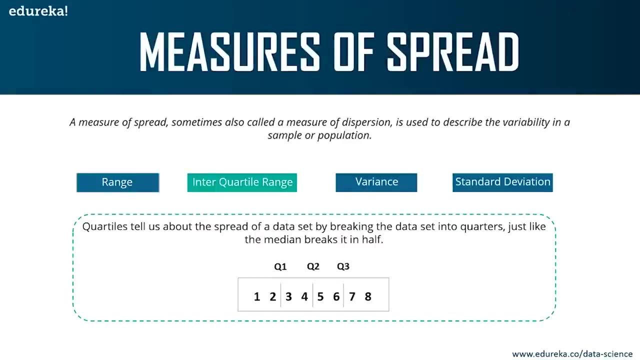 are. the range can be calculated as shown in this formula. So you basically going to subtract the maximum value in your data set from the minimum value in your data set. That's how you calculate the range of the data. All right. Next we have interquartile range. 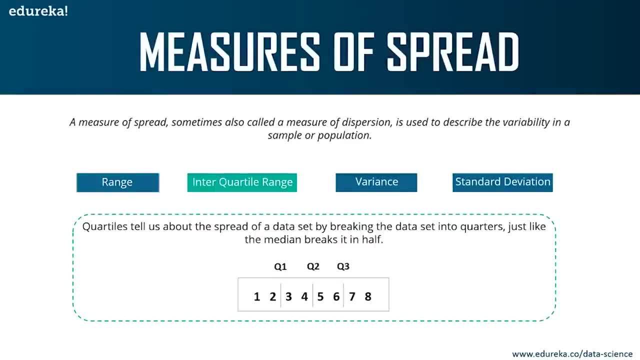 So before we discuss interquartile range, let's understand what a quartile is. All right, So quarter is basically tell us about the spread of a data set by breaking the data set into different quarters. Okay, just like how the median breaks the data into two parts: the 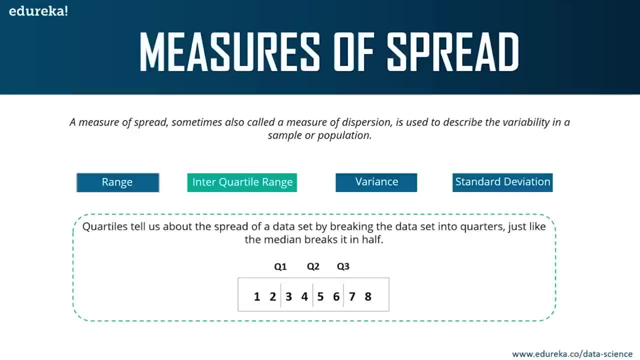 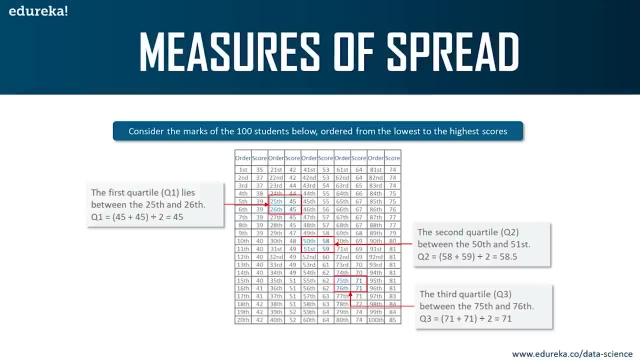 quartile will break it into different quarters. So to better understand how quartile and interquartile are calculated, Let's look at a small example Now. this data set basically represents the marks of hundred students, ordered from the lowest to the highest course. 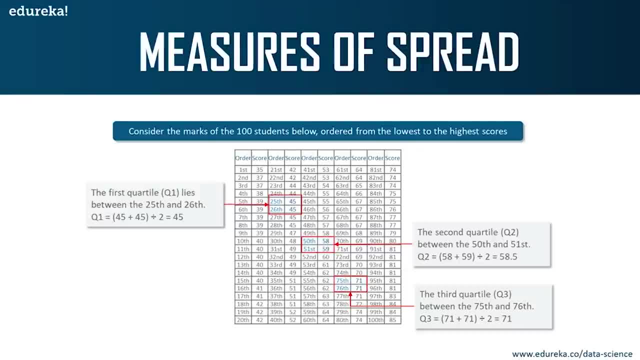 All right. So the quartiles lie in the following ranges and the first quartile, which is also known as q1. It lies between the 25th and 26th observation, All right. So if you look at this, I've highlighted the 25th and the 26th observation. 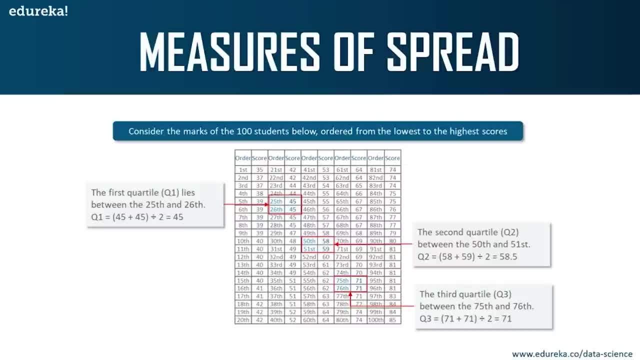 So how you can calculate q1, or first quartile, is by taking the average of these two values. All right, since both the values are 45, when you add them up and divide them by two, you'll still get 45.. Now the second quartile, or q2, is between the 50th and the 51st. 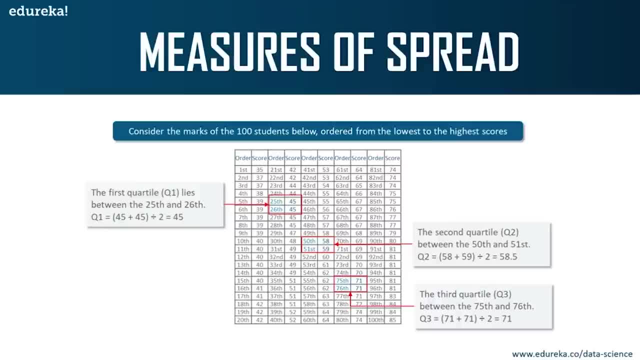 observation. So you're going to take the average of 58 and 59 and you'll get a value of 58.5.. Now this is my second quarter. The third quartile, or q3, is between the 75th and the 76th observation. 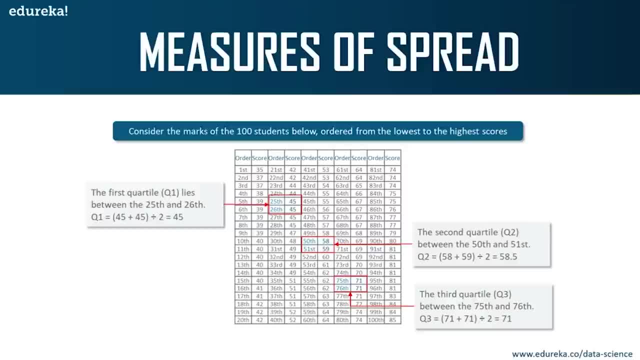 Here again, we'll take the average of the two values, which is the 75th value and the 76th value, All right, and you'll get a value of 71.. All right, So, guys, this is exactly how you calculate the different quartiles. 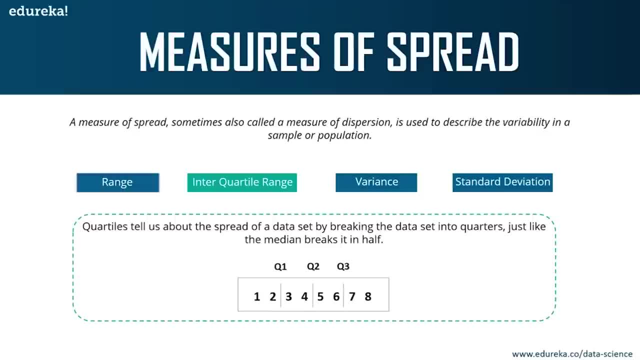 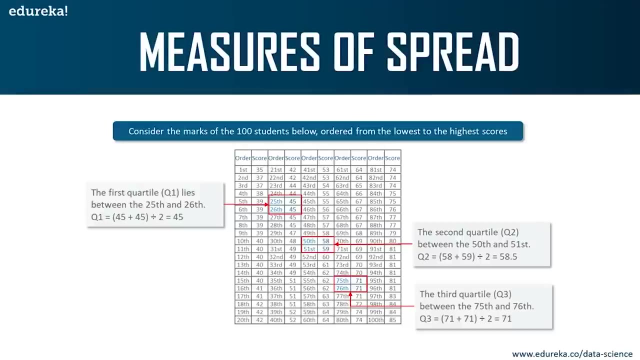 Okay, just like How the median breaks the data into two parts, The quartile will break it into different quarters. So to better understand how quartile and interquartile are calculated, Let's look at a small example Now. this data set basically represents the marks of hundred students, ordered from the lowest to the highest course. 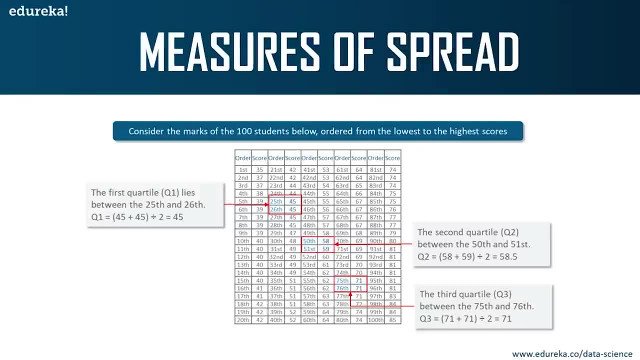 All right, so the quartiles lie in the following ranges. Now the first quartile, which is also known as Q1. it lies between the 25th and the 26th observation. All right, So if you look at this, I've highlighted the 25th and the 26th observation. 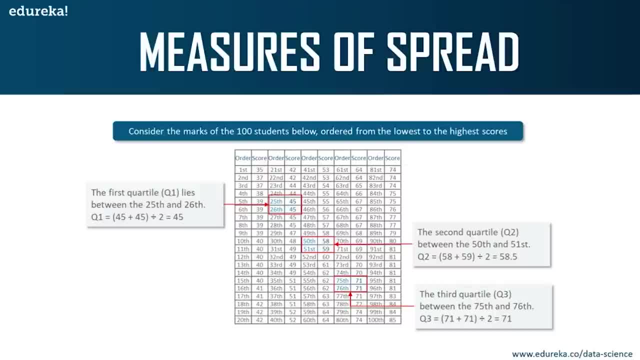 So how you can calculate Q1, or first quartile, is by taking the average of these two values. All right, since both the values are 45, when you add them up and divide them by 2, you'll still get 45.. Now the second quartile, or Q2, is between the 50th and the 51st observation. 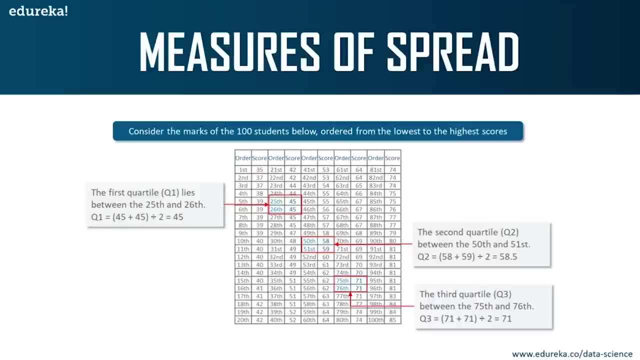 So you're going to take the average of 58 and 59 and you'll get a value of 58.. Now this is my second quarter. The third quartile, or Q3, is between the 75th and the 76th observation. 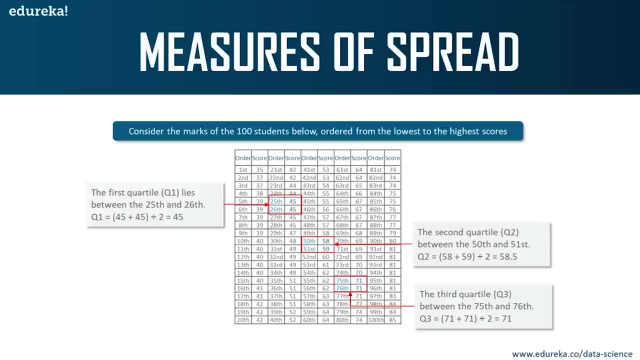 Here again, we'll take the average of the two values, which is the 75th value and the 76th value, All right, and you'll get a value of 71.. All right, So, guys, this is exactly how you calculate the different quartiles. 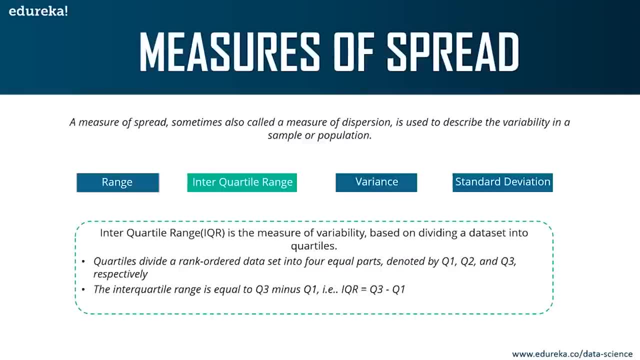 Now let's look at what is interquartile range. So IQR, or the interquartile range, is a measure of variability Based on dividing a data set into quartiles. Now the interquartile range is calculated by subtracting the Q1 from Q3.. 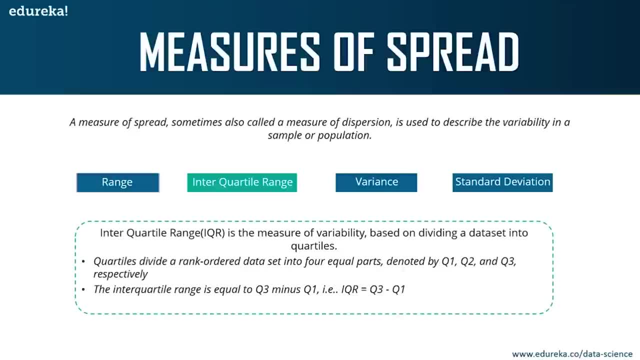 So, basically, Q3 minus Q1 is your IQR. So your IQR is your Q3 minus Q1.. All right, Now this is how each of the quartiles are. Each quartile represents a quarter, which is 25%. 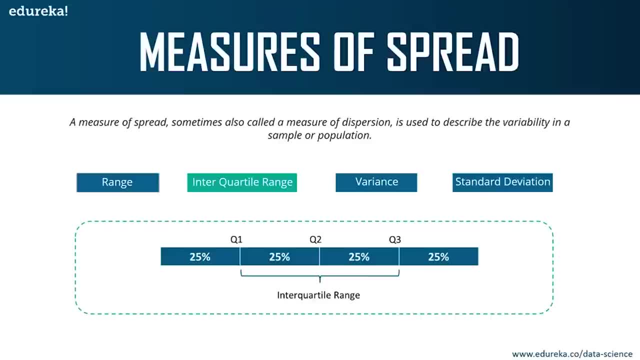 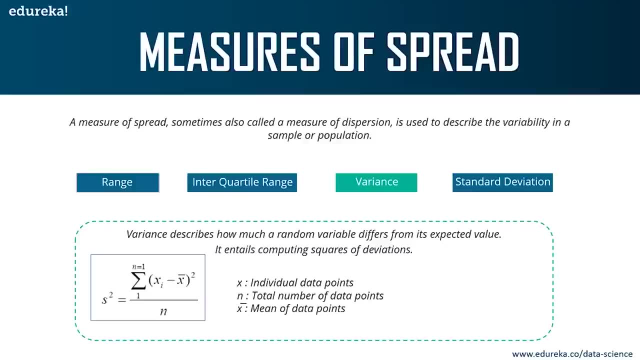 All right. So, guys, I hope all of you are clear with interquartile range and what are quartiles? Now let's look at variance. Now, variance is basically a measure that shows how much a random variable differs from its expected value. 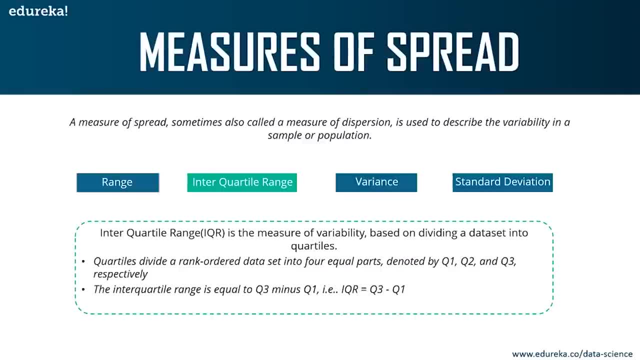 Now let's look at what is interquartile range. So IQR, or the interquartile range, is a measure of variability based on dividing a data set into quartiles. Now the interquartile range is calculated by subtracting the q1 from: 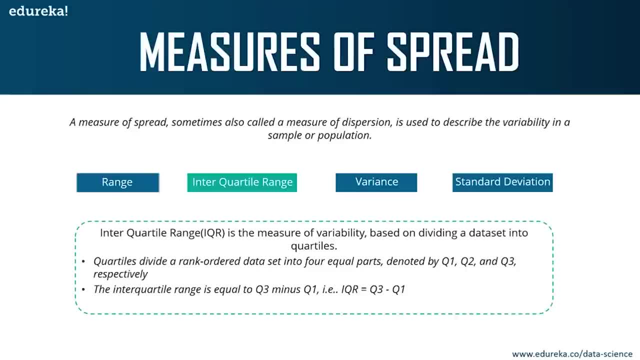 q3.. So basically, q3 minus q1 is your IQR. So your IQR is your q3 minus q1.. All right, Now. this is how each of the quartiles are. each quartile represents a quarter, which is 25%. 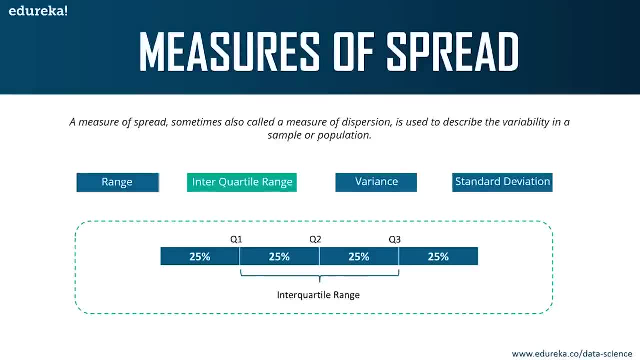 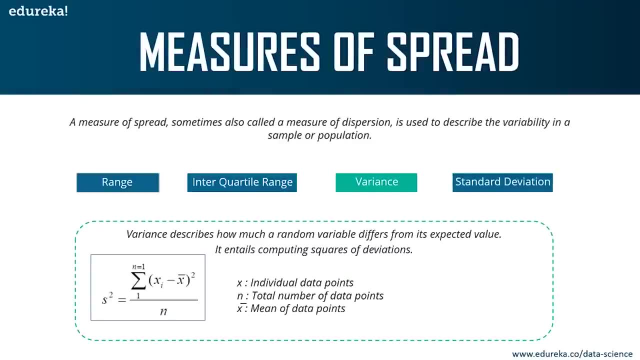 All right. So, guys, I hope all of you are clear with interquartile range and what are quartiles? Now let's look at variance. Now, variance is basically a measure That shows how much a random variable differs from its expected value. 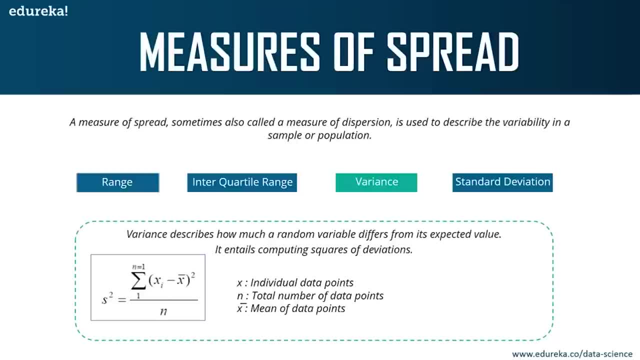 Okay, It's basically the variance in any variable. Now variance can be calculated by using this formula right here: X basically represents any data point in your data set, N is the total number of data points in your data set And X bar is basically the mean of data points. 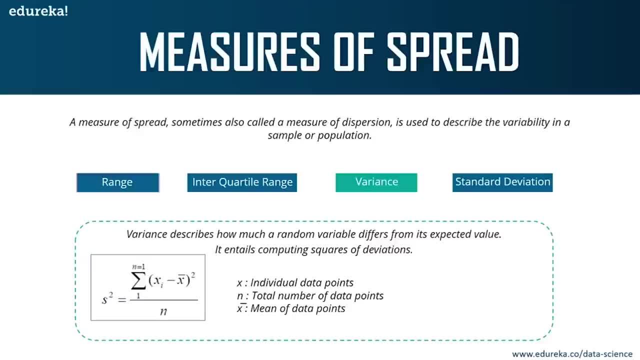 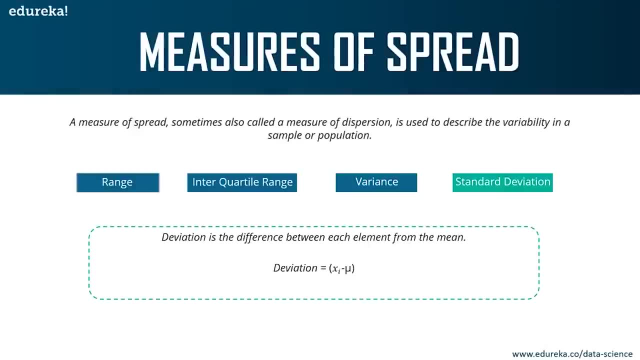 All right, This is how you calculate variance. Variance is basically a computing the squares of deviations. Okay, That's why it says S squared there. Now let's look at what is deviation. Deviation is just the difference between each element from the mean. 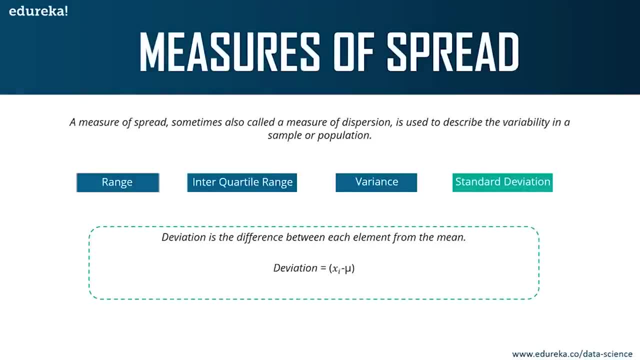 Okay, So it can be calculated by using this simple formula, where X- I- basically represents a data point and mu is the mean of the population. All right, This is exactly how you calculate deviation. Now, population variance and sample variance are very specific to. 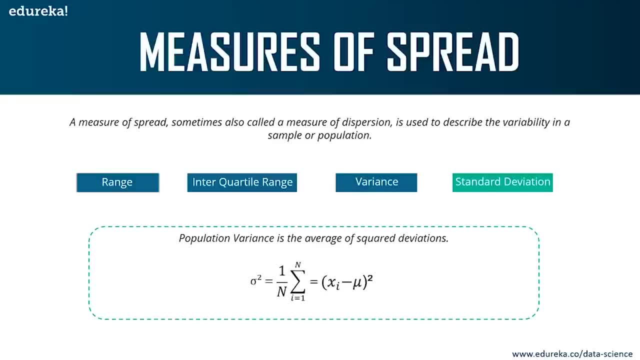 whether you're calculating the variance in your population data set or in your sample data set. That's the only difference between population and sample variance. So the formula for population variance is pretty explanatory. So X- I is basically each data point, mu is the mean of the population. 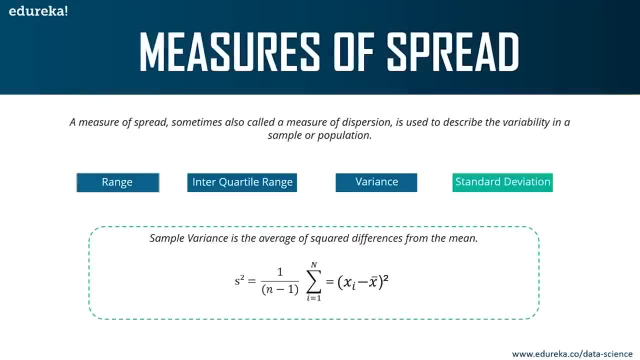 and is the number of samples in your data set. All right, Now let's look at sample variance. Now, sample variance is the average of squared differences from the mean. All right, Your X I is any data point or any sample in your data set. X bar is the mean. 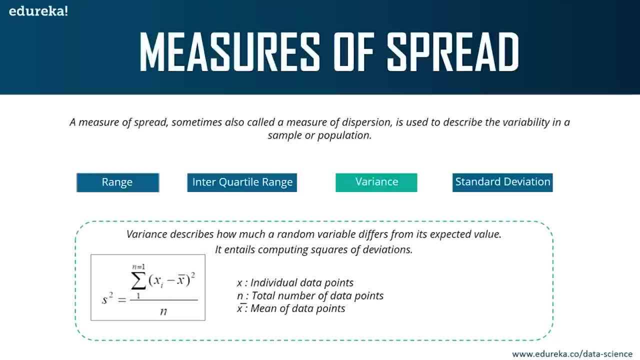 Okay, it's basically the variance in any variable. Now variance can be calculated by using this formula right here: X basically represents any data point in your data set, N is the total number of data points in your data set And X bar is basically the mean of data points. 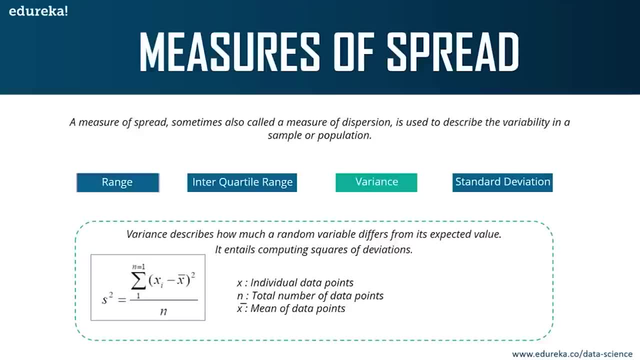 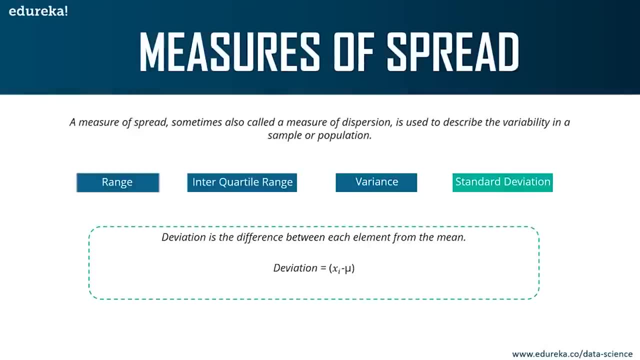 All right, This is how you calculate variance. Variance is basically computing the squares of deviations. Okay, that's why it says S squared there. Now let's look at what is deviation. Deviation is just the difference between each element from the mean. 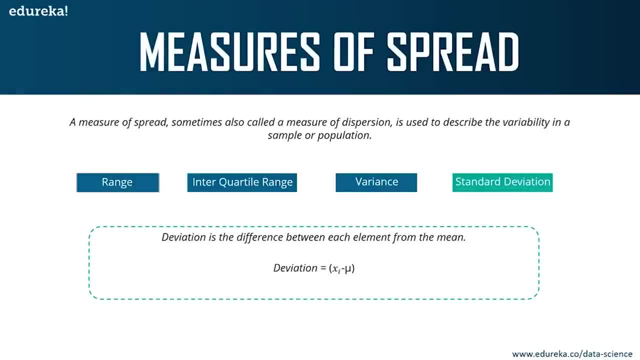 Okay, so it can be calculated by using this simple formula, where X- I basically represents a data point and mu is the mean of the population. All right, This is exactly how you calculate deviation. Now, population variance and sample variance are very specific to whether you're. 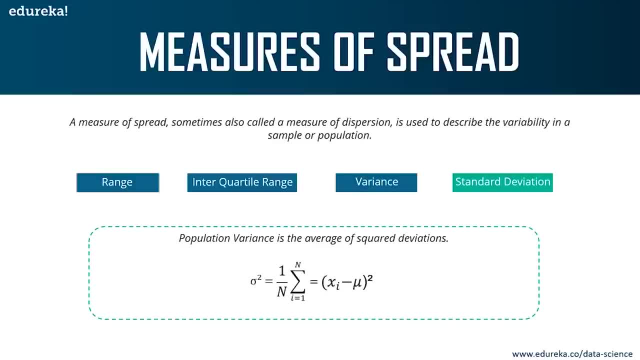 calculating the variance In your population data set or in your sample data set. That's the only difference between population and sample variance. So the formula for population variance is pretty explanatory. So X- I is basically each data point, mu is the mean of the population. 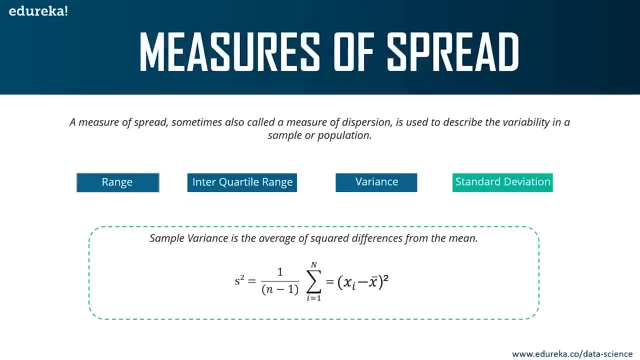 and is the number of samples in your data set. All right, Now let's look at sample variance. Now, sample variance is the average of squared differences from the mean. All right, your X I is any data point or any sample in your data set. 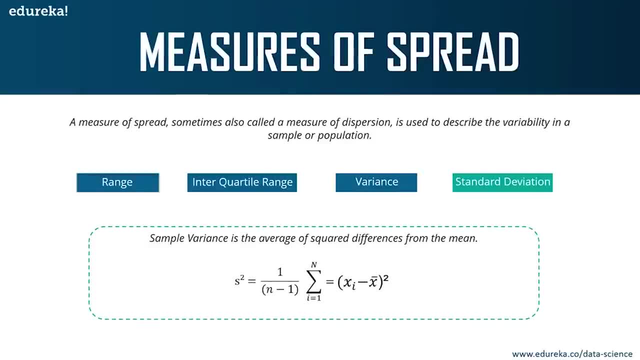 X bar is the mean of your sample. All right, it's not the mean of your population, It's the mean of your sample. And if you notice n- here is a smaller n- it's the number of data points in your sample. 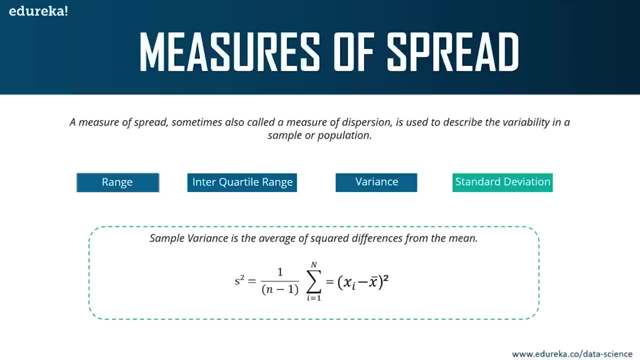 And this is basically the difference between sample and population variance. I hope that is clear. Coming to standard deviation is the measure of dispersion of a set of data from its mean. All right, so it's basically the deviation from your mean. That's what standard deviation is. 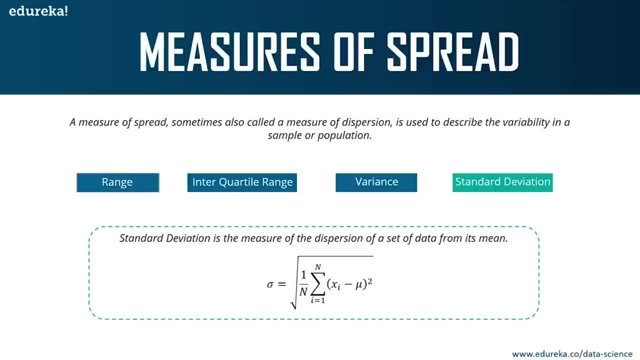 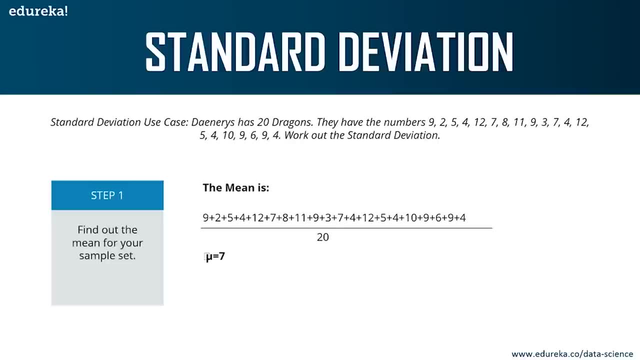 Now to better understand, Understand how the measures of spread are calculated, Let's look at a small use case. So let's say Daenerys has 20 dragons. They have the numbers 9, 2, 5, 4 and so on, as shown on the screen. 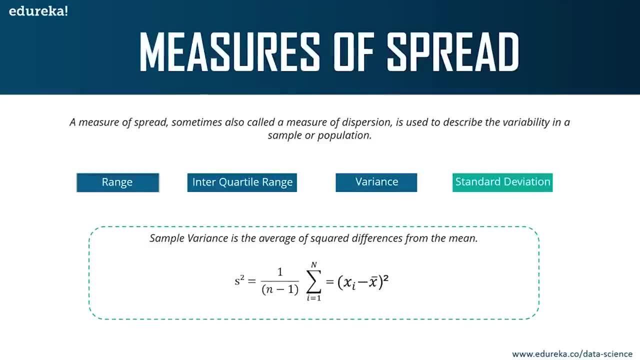 of your sample. All right, It's not the mean of your population, It's the mean of your sample And if you notice n, here is a smaller n, It's a number of data points in your sample And this is basically the difference between sample and population variance. 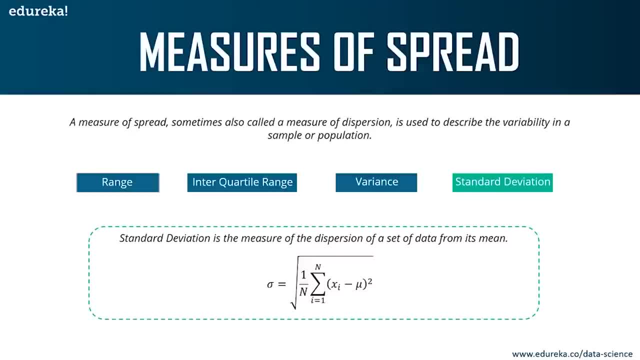 I hope that is clear. Coming to standard deviation is the measure of dispersion of a set of data from its mean. All right, So it's basically the deviation from your mean. That's what standard deviation is. Now to better understand how the measures of spread are calculated. 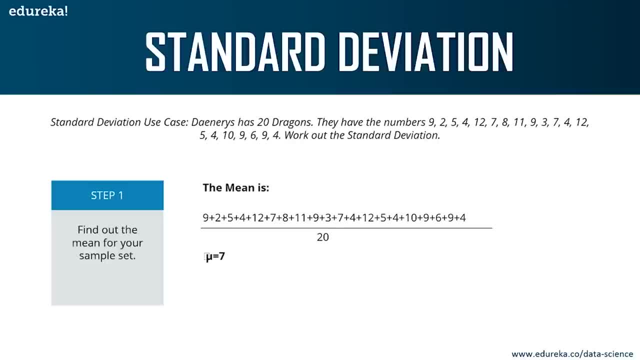 Let's look at a small use case. So let's say Daenerys has 20 dragons. They have the numbers 9, 2, 5, 4 and so on, as shown on the screen. What you have to do is you have to work out the standard deviation. 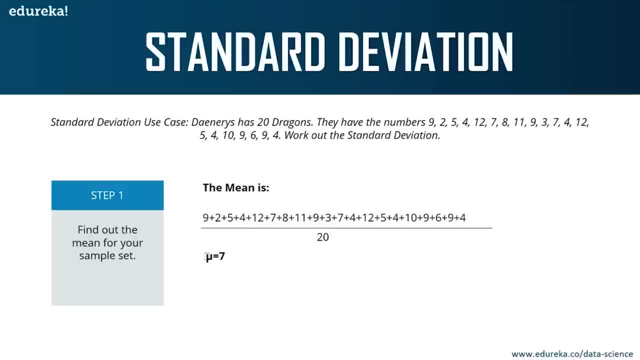 All right. In order to calculate the standard deviation You need to know the mean right. So first you're going to find out the mean of your sample set. So how do you calculate the mean? you add all the numbers in your data set and divided by the total number of samples in your data set. 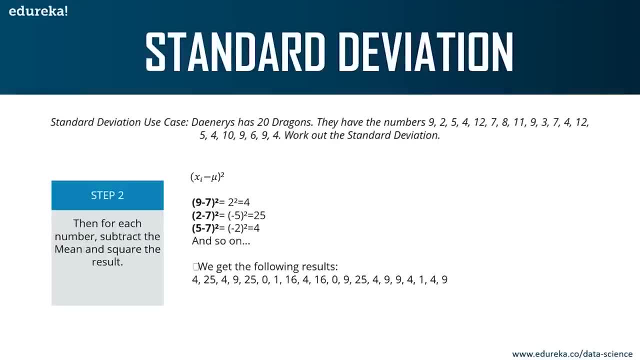 So you get a value of 7 here. Then you calculate the RHS of your standard deviation formula, All right. So from each data point you're going to subtract the mean and you're going to square that, All right. So when you do that you'll get the following result: 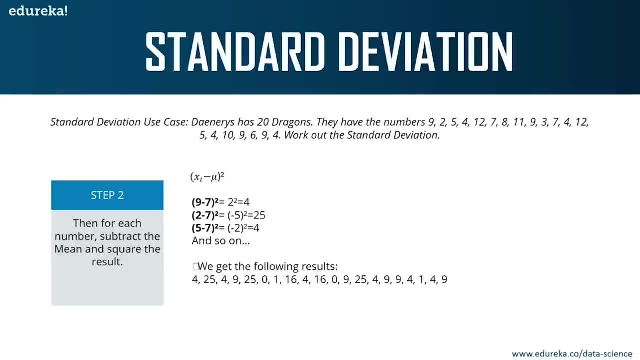 You'll basically get this: 4, 25, 4, 9, 25 and so on. So finally you will just find the mean of these squared differences. All right, So your standard deviation will come up to 2.983 once you take the square. 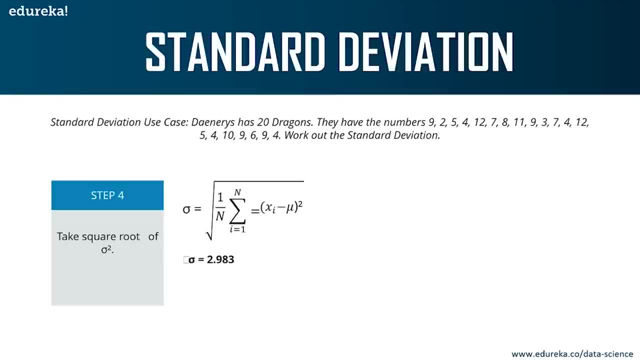 root. So, guys, is pretty simple. It's a simple mathematic technique. All you have to do is you have to substitute the values in the formula. All right, I hope this was clear to all of you. Now let's move on and discuss the next topic, which is information gain. 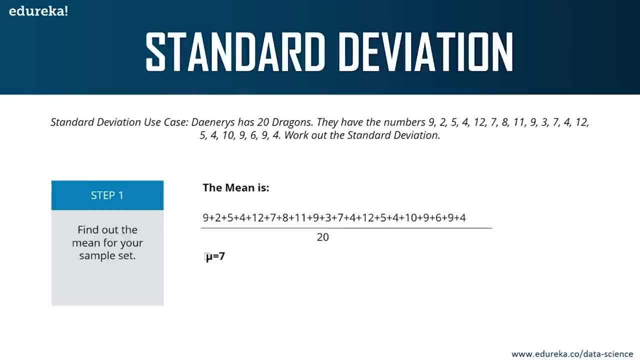 What you have to do is you have to work out the standard deviation. All right, in order to calculate the standard deviation, you need to know the mean, right? So first you're going to find out the mean of your sample set. So how do you calculate the mean? you add all the numbers in your data set and 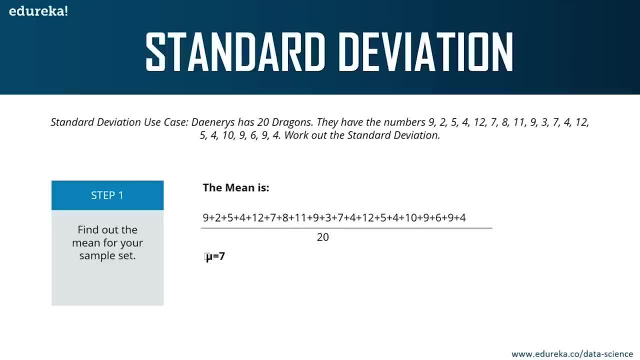 divided by the total number of samples in your data set. So you get a value of 7 here. Then you calculate the RHS of your standard deviation formula. All right, So from each data point you're going to subtract the mean and you're going to square that. 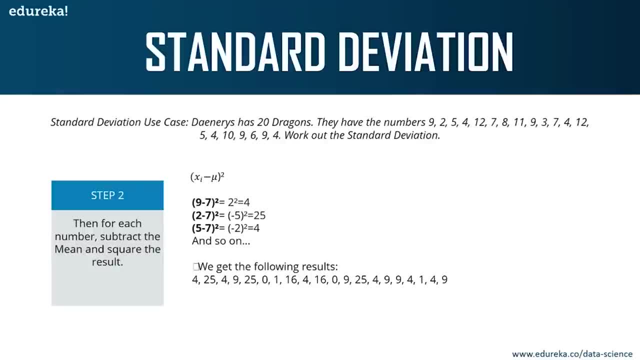 All right. So when you do that, you'll get the following result: You'll basically get this: 425, 49, 25 and so on. So finally, you will just find the mean of these squared differences. All right, so your standard deviation will come up to 2.. 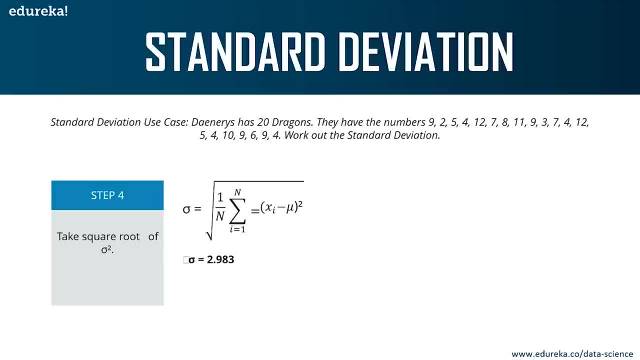 Point 983 once you take the square root. So, guys, is pretty simple. It's a simple mathematic technique. All you have to do is you have to substitute the values in the formula. All right, I hope this was clear to all of you. 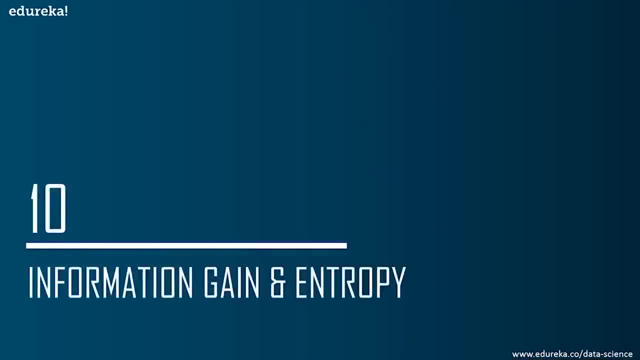 Now let's move on and discuss the next topic, which is information gain and entropy. Now, this is one of my favorite topics in statistics. It's very interesting, and this topic is mainly involved in machine learning algorithms like decision trees and random forest. 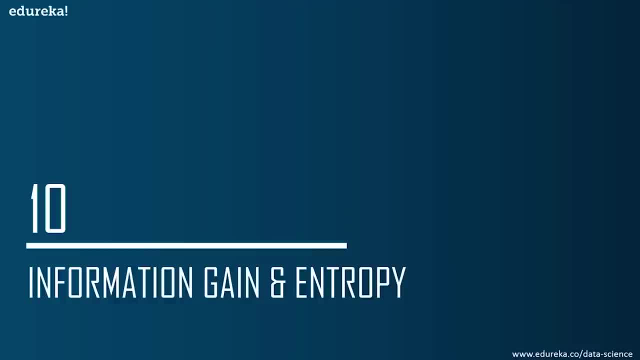 All right, it's very important for you to know how information gain and entropy really work and why they're so essential in building machine learning models. We'll focus on the statistic parts of information gain and entropy And after that we'll discuss a use case and see how information gain and entropy is used in 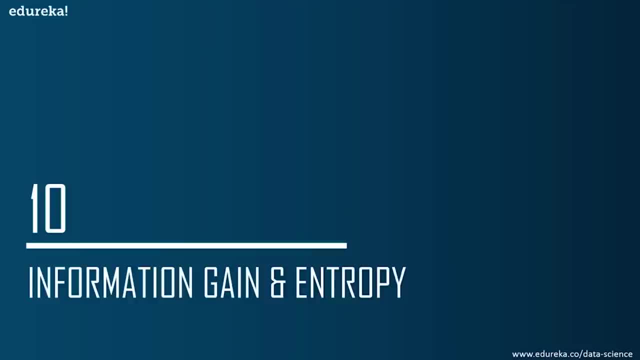 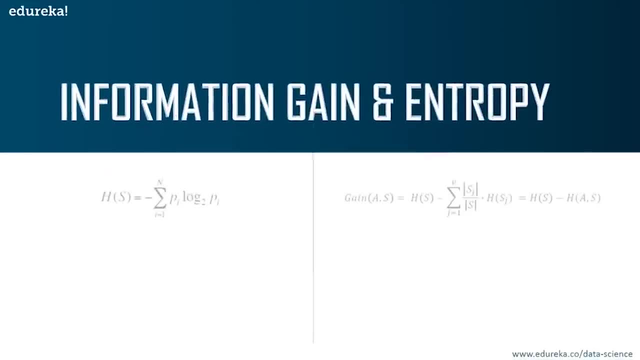 decision trees. So for those of you who don't know what a decision tree is, it is basically a machine learning algorithm. You don't have to know anything about this. I'll explain everything in depth, So don't worry. Now let's look at. 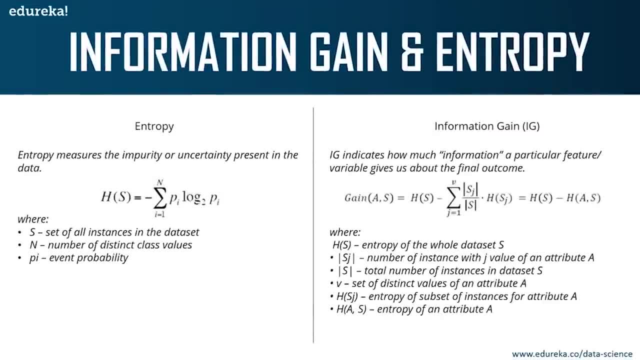 What exactly entropy and information gain is. Now, guys, entropy is basically the measure of any sort of uncertainty that is present in the data. All right, so it can be measured by using this formula. So your S is the set of all instances in the data set, or all the data items in 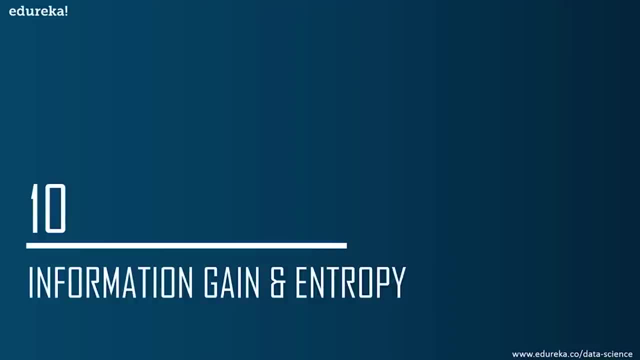 and entropy. Now, this is one of my favorite topics in statistics. It's very interesting, and this topic is mainly involved in machine learning algorithms like decision trees and random Forest. All right, It's very important for you to know How information gain and entropy really work and why they're so essential. 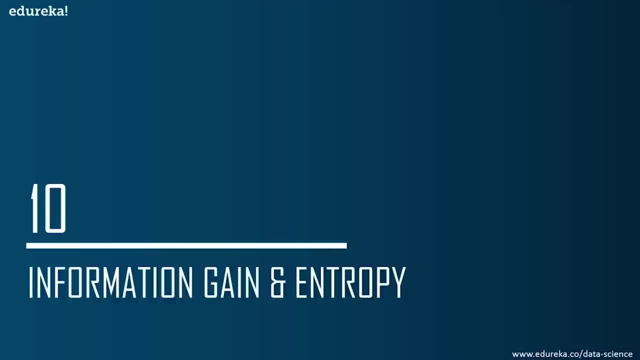 in building machine learning models. We'll focus on the statistic parts of information gain and entropy and after that we'll discuss a use case and see how information gain and entropy is used in decision trees. So for those of you who don't know what a decision tree is, it is basically 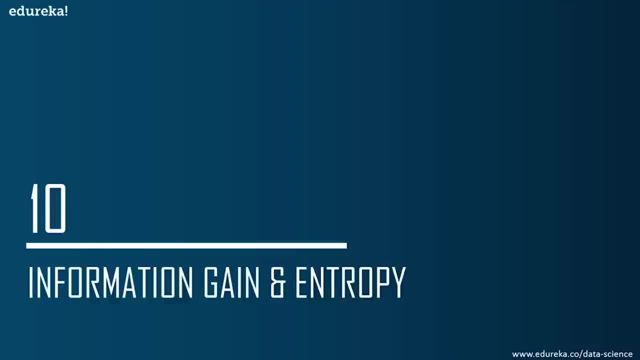 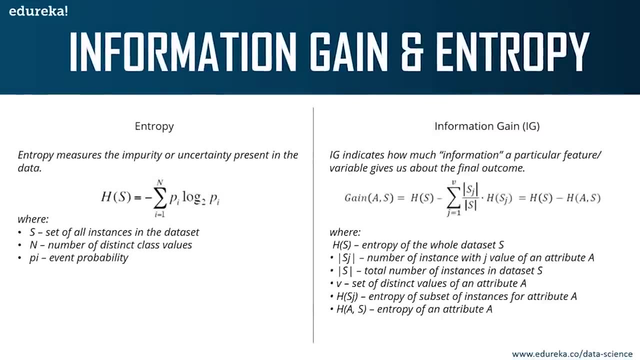 a machine learning algorithm. You don't have to know anything about this. I'll explain everything in depth, So don't worry. now Let's look at what exactly entropy and information gain Is. Now, guys, entropy is basically the measure of any sort of uncertainty. that 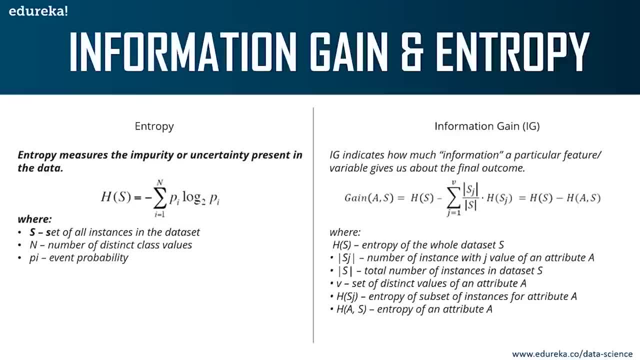 is present in the data, All right, so it can be measured by using this formula. So your S is the set of all instances in the data set or all the data items in the data set, and is the different type of classes in your data set. 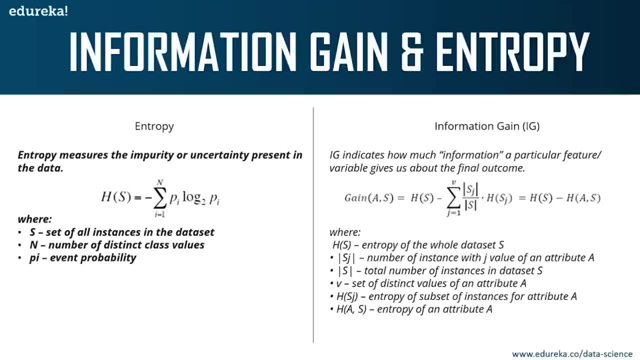 P, I is the event probability. Now, this might seem a little confusing to y'all, But when we go through the use case you will understand all of these terms even better. All right, coming to information gain. as the word suggests, information gain indicates how much information a particular feature or a particular 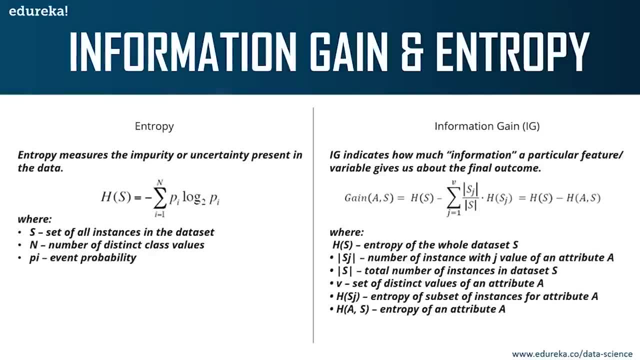 variable gives us about the final outcome. Okay, it can be measured by using this formula. So again here. hedge of S is the entropy of the whole data set: S, S, J is the number of instances with the J value of an attribute. a S is 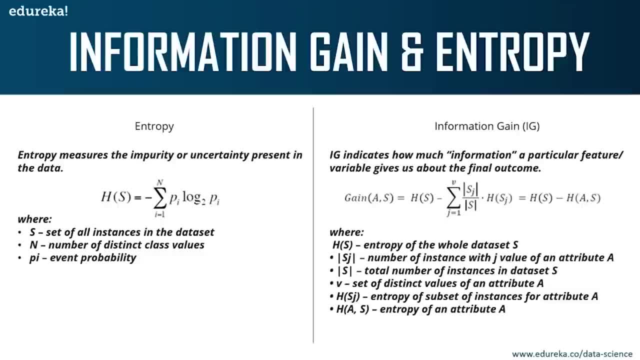 the total number of instances in the data set. V is the set of distinct values of an attribute A, H of S, J is the entropy of subset of instances, and H of a comma S is the entropy of an attribute a. even though this seems confusing, I'll clear out the 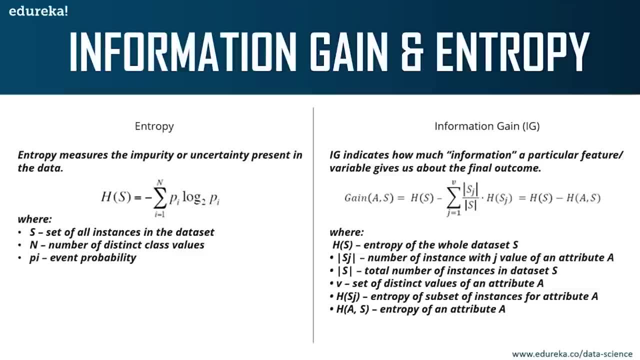 confusion. All right, let's discuss a small problem statement where we'll understand how information gain and entropy is used to study the significance of a model. So, like I said, information gain and entropy are very important statistical measures that let us understand the significance of a problem. 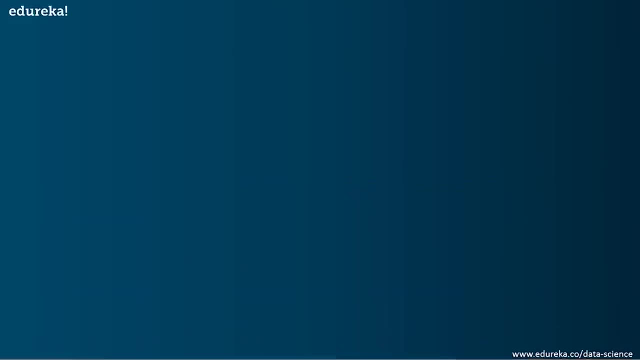 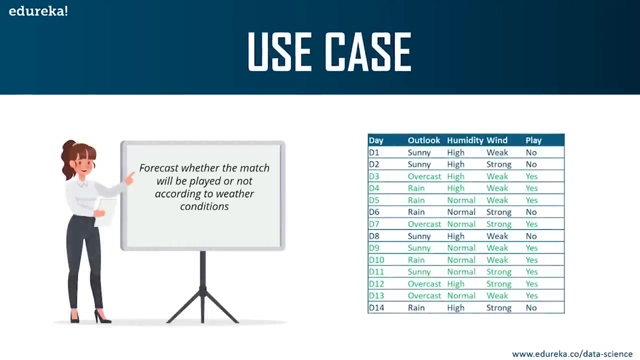 Predictive model. Okay, to get a more clear understanding, Let's look at a use case. All right, Now suppose we're given a problem statement. All right. The statement is that you have to predict whether a match can be played or not by studying the weather conditions. 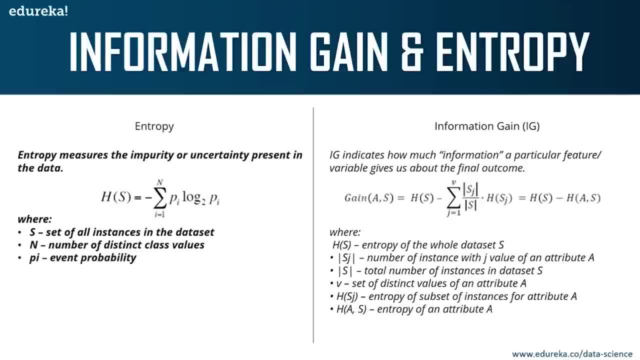 the data set and is the different type of classes in your data set. PI is the event probability. Now, this might seem a little confusing to y'all, but when we go through the use case you'll understand all of these terms even better. 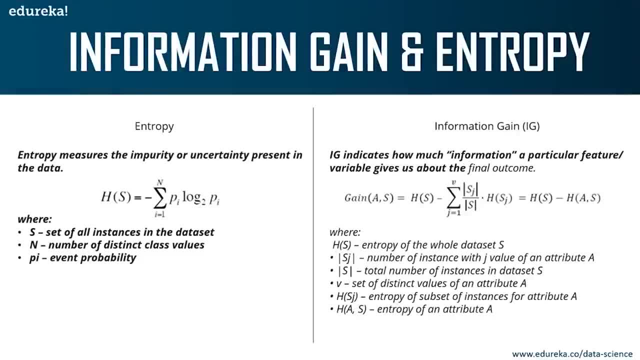 All right, coming to information gain. as the word suggests, information gain indicates how much information a particular feature or a particular variable gives us about the final outcome. Okay, it can be measured by using this formula. So, again, your hedge of S is the entropy of the whole data set. 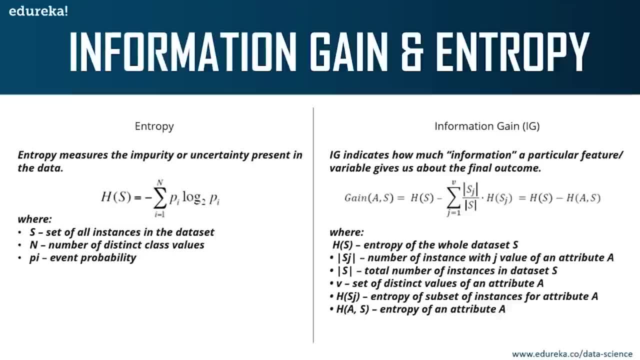 S, S. J is the number of instances with the J value of an attribute A. S is the total number of instances in the data set. V is the set of distinct values of an attribute A, H of S, J is the entropy of subset of instances and H of A. 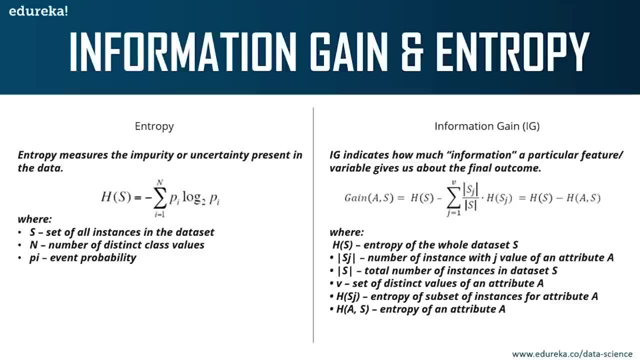 S is the entropy of an attribute A. Even though this seems confusing, I'll clear out the confusion. All right, let's discuss a small problem statement where we'll understand how information gain and entropy is used to study the significance of a model. 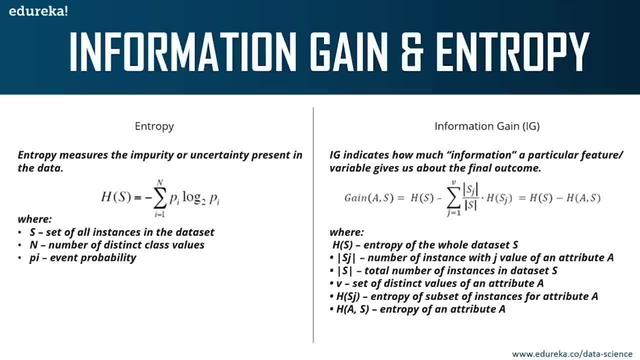 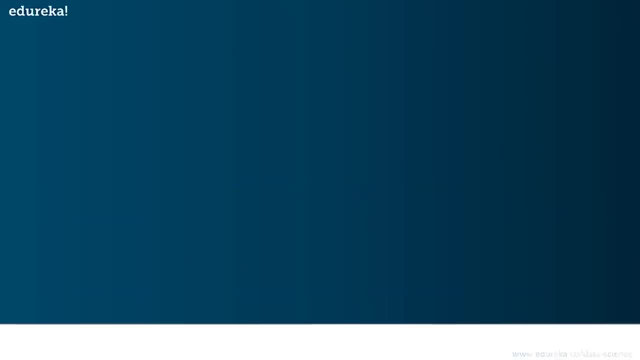 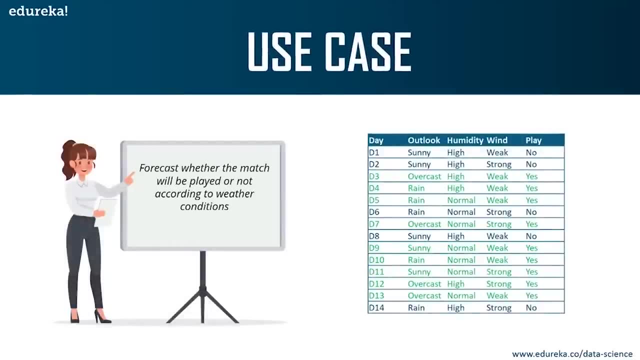 So, like I said, information gain and entropy are very important statistical measures That let us understand the significance of a predictive model. Okay, to get a more clear understanding, Let's look at a use case. All right, Now suppose we're given a problem statement. 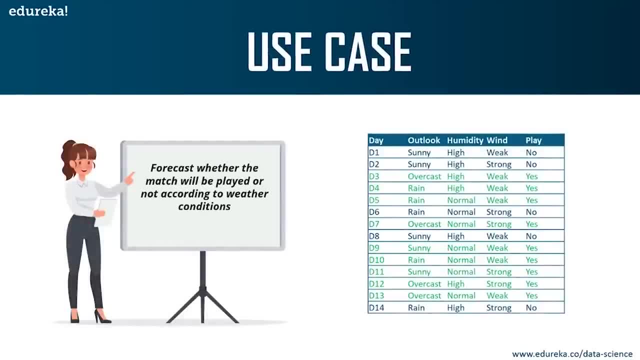 All right. the statement is that you have to predict whether a match can be played or not by studying the weather conditions. So the predictor variables here are outlook, humidity, wind day is also a predictor variable. The target variable is basically play. 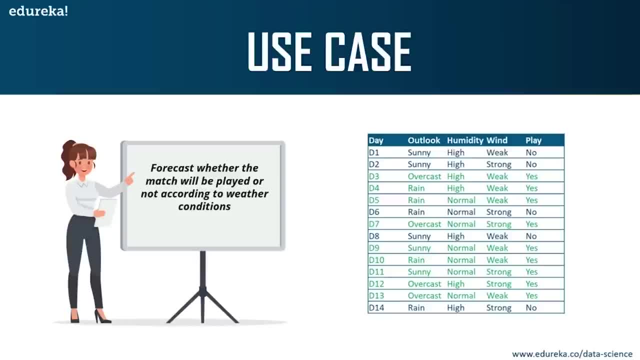 All right, the target variable is the variable that you're trying to predict. Okay, Now, the value of the target variable will decide whether or not a game can be played. All right, So that's why the play has two values. 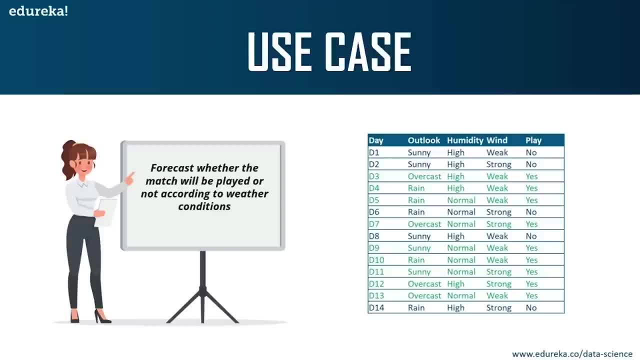 It has no and yes, no meaning that the weather conditions are not good And therefore you cannot play the game. Yes, meaning that the weather conditions are good and suitable for you to play the game, All right. So that was a problem statement. 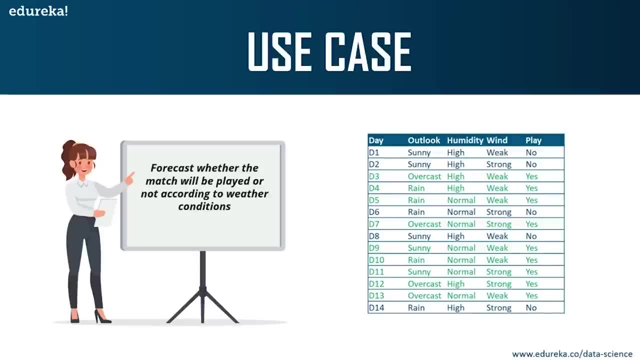 So the predictor variables here are: outlook, humidity. wind day is also a predictor variable. The target variable is basically play. All right, the target variable is the variable that you're trying to predict. Okay, Now, the value of the target variable will decide whether or not a game can. 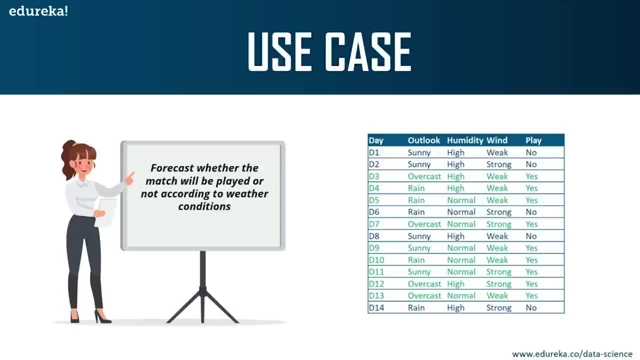 be played All right. So that's why the play has two values. It has no and yes. no meaning that the weather conditions are not good and therefore you cannot play the game. Yes, meaning that the weather conditions are good and suitable for you to. 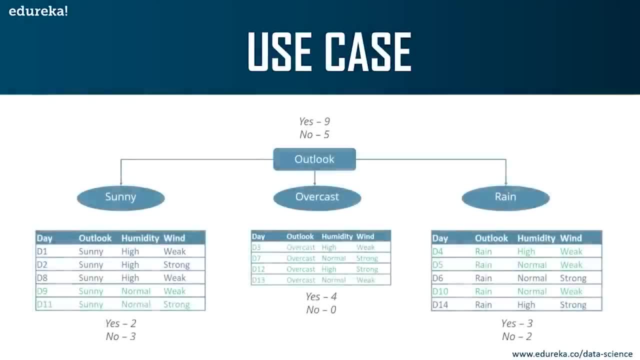 play the game. All right, So that was a problem statement. I hope the problem statement is clear to all of you now. to solve such a problem We make use of something known as decision trees. So guys Think of an inverted tree and each branch of the tree denotes some decision. 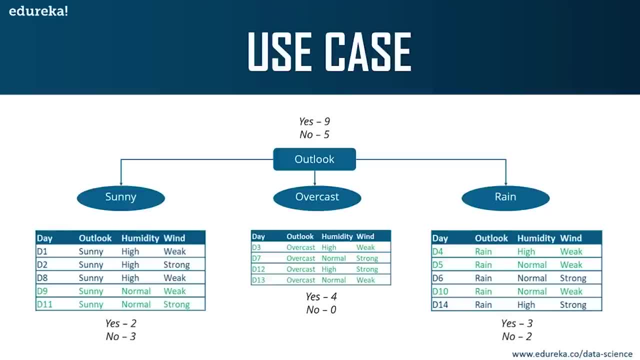 All right. each branch is known as the branch node, and at each branch node You're going to take a decision in such a manner that you will get an outcome at the end of the branch. All right Now. this figure here basically shows that, out of 14 observations, nine: 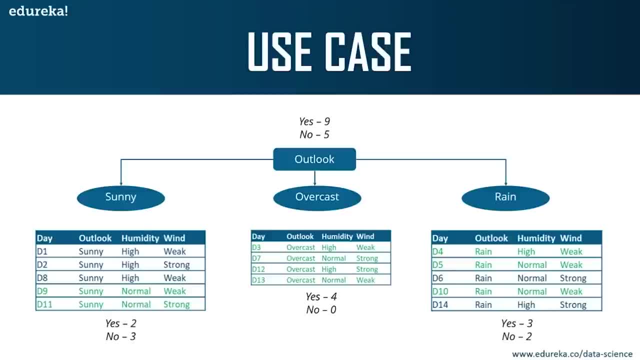 observations result in a yes, meaning that out of 14 days, the match can be played only on nine days. All right, So here, if you see, on day 1, day 2, day 8, day 9 and day 11, the outlook has been: 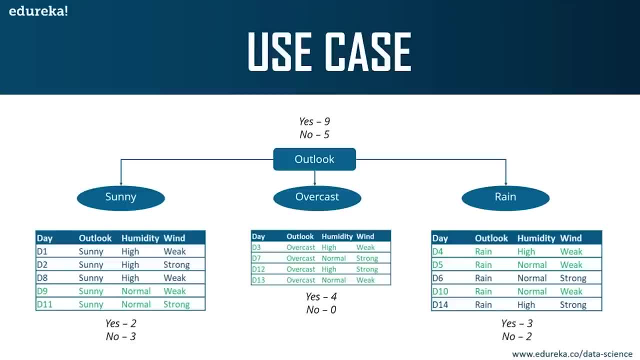 sunny, All right. So basically, we're trying to cluster our data set depending on the outlook. So, when the outlook is sunny, this is our data set. when the outlook is overcast, This is what we have, and when the outlook is rain, this is what we have. 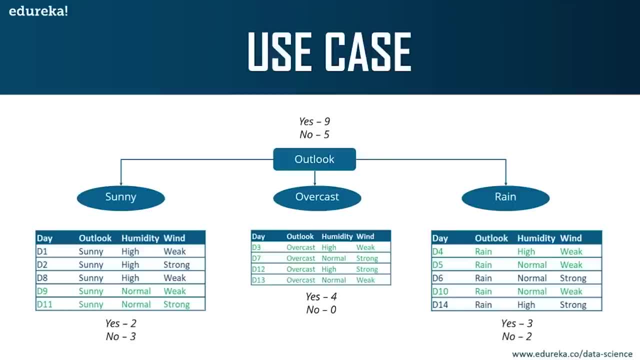 All right. So when it is sunny, we have two yeses and three noes. Okay, when the outlook is overcast, We have all four As yeses, meaning that on the four days when the outlook was overcast, we can. 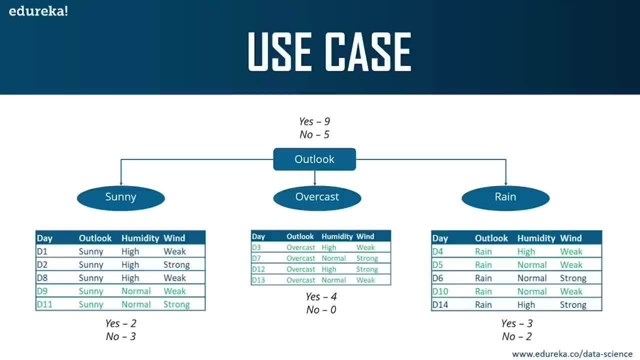 play the game. All right. Now, when it comes to rain, we have three yeses and two noes, All right. So, if you notice, here the decision is being made by choosing the outlook variable as the root node. Okay, So the root node is basically the topmost node in a decision tree. 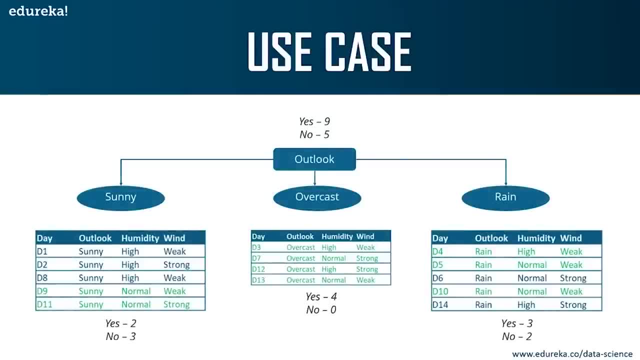 I hope the problem statement is clear to all of you. now, to solve such a problem We may Use of something known as decision trees. So guys think of an inverted tree and each branch of the tree denotes some decision. All right, each branch is known as the branch node and at each branch node 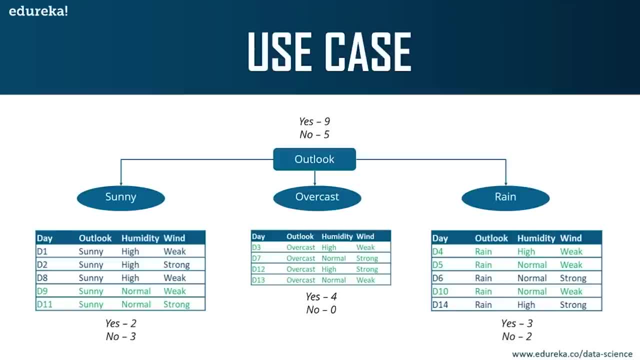 you're going to take a decision in such a manner that you will get an outcome at the end of the branch. All right Now. this figure here basically shows that out of 14 observations, nine observations result in a yes, meaning that out of 14 days. 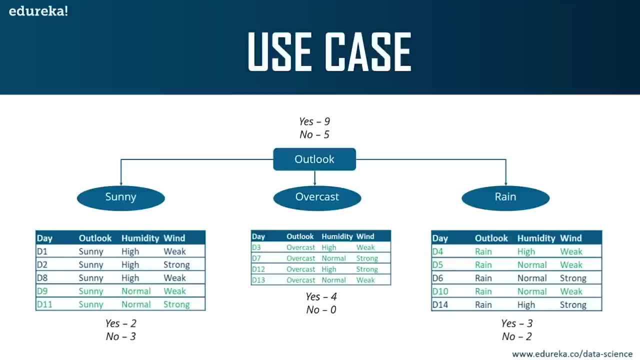 the match can be played only on nine days, All right. So here, if you see, on day 1, day 2, day 8, day 9 and day 11, the outlook has been sunny, All right. So basically, we're trying to cluster our data set depending on the outlook. 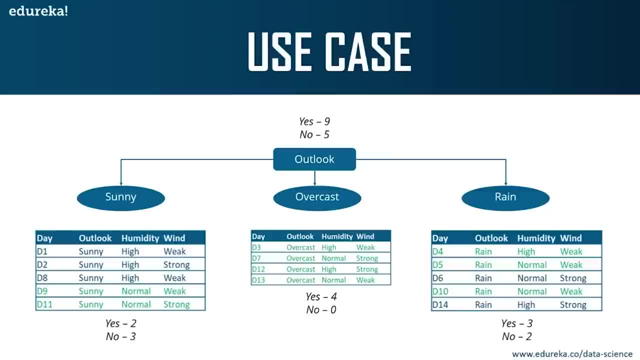 So when the outlook is sunny, this is our data set. when the outlook is overcast, This is what we have, and when the outlook is rain, this is what we have. All right, So when it is sunny, we have two yeses and three nos. 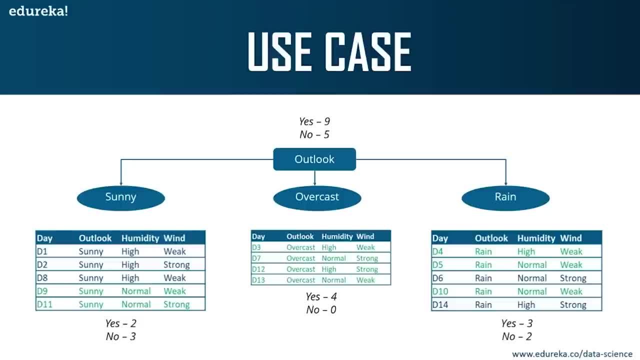 Okay, when the outlook is overcast, we have all four as yeses, meaning that on the four days when the outlook was overcast, we can play the game All right. Now, when it comes to rain, we have three yeses and two nos. 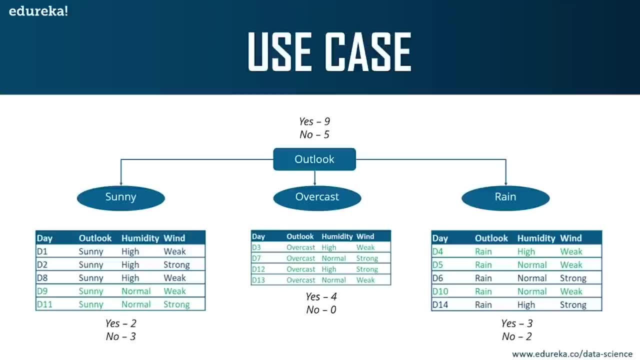 All right. So, if you notice, here the decision is being made by choosing the outlook variable as the root node. Okay, So the root node is basically the topmost node in a decision tree. Now, what we've done here is we've created a decision tree that starts with the. 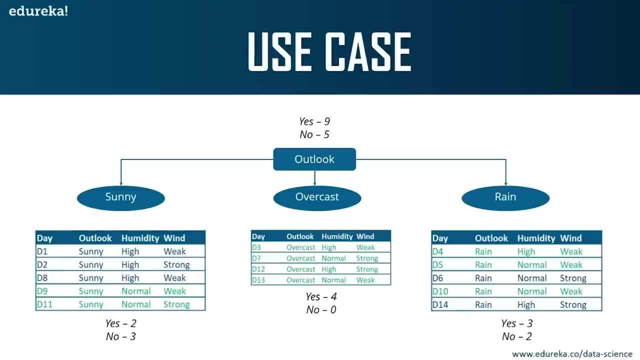 outlook node. All right, then you're splitting the decision tree further, depending on other parameters like sunny, overcast and rain. All right, Now, like we know, that outlook has three values- sunny, overcast and rain- So let me explain this in a more in-depth manner. 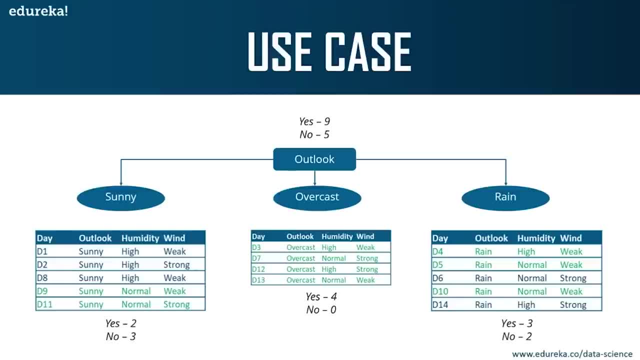 Okay. So what you're doing here is you're making the decision tree by choosing the outlook variable at the root node. The root node is basically the topmost node in a decision tree. Now the outlook node has three branches Coming out from it. 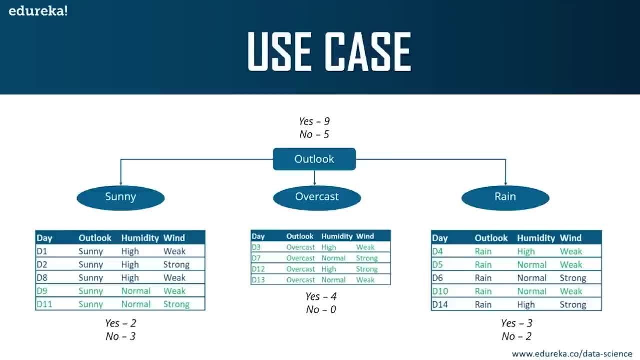 Now, what we've done here is we've created a decision tree that starts with the outlook node. All right, then you're splitting the decision tree further, Depending on other parameters like sunny, overcast and rain. All right, Now, like we know, that outlook has three values: sunny, overcast and rain. 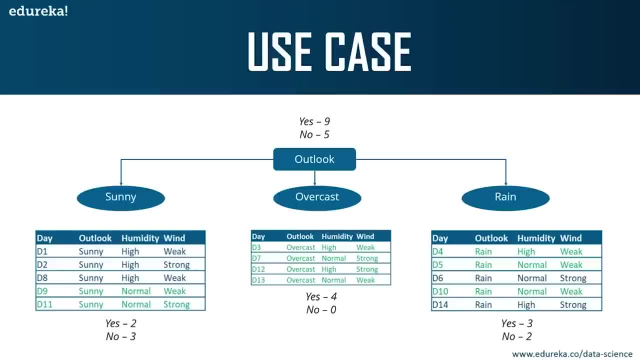 So let me explain this in a more in-depth manner. Okay, So what you're doing here is you're making the decision tree by choosing the outlook variable at the root node. The root node is basically the topmost node in a decision tree. 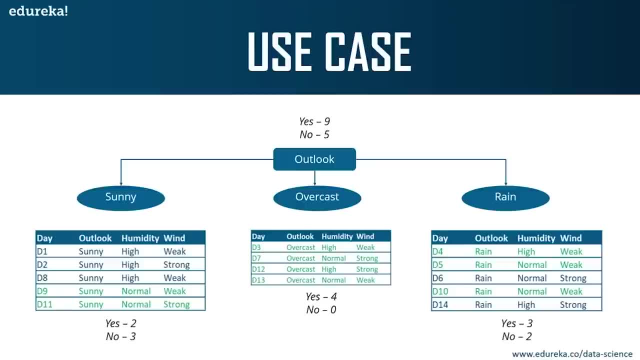 Now the outlook node has three branches coming out from it, which is sunny, overcast and rain. So basically, outlook can have three values: either It can be sunny, It can be overcast or it can be rainy. Okay, Now these three values are assigned to the immediate branch nodes and for 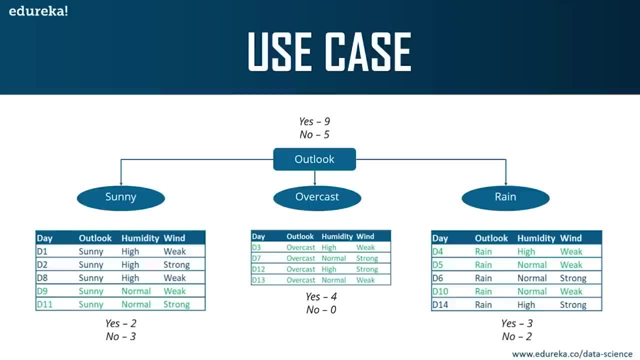 each of these values, the possibility of play is equal to yes is calculated, So the sunny and the rain branches will give you an impure output, meaning that there is a mix of yes and no right. There are two yeses here, three noes here. 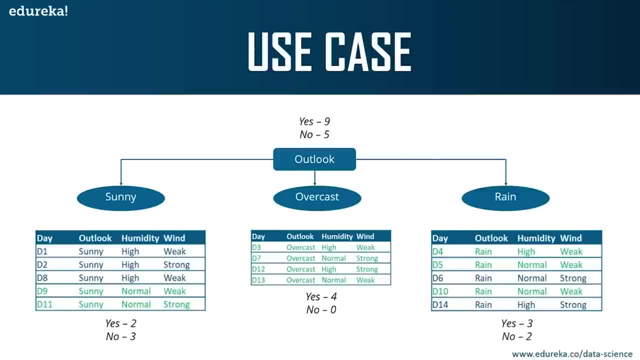 There are three yeses here and two noes over here, But when it comes to the overcast variable, it results in a hundred percent pure subset. All right, this shows that the overcast variable will result in a definite and certain output. 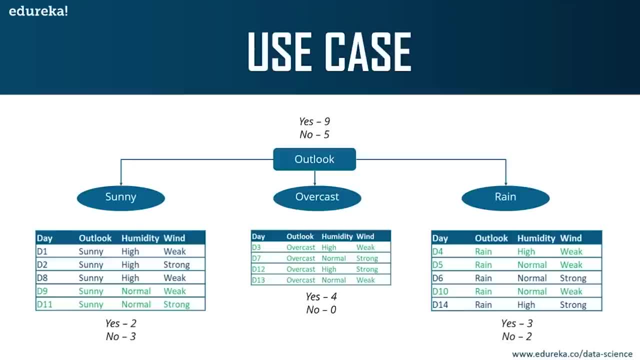 This is exactly what entropy is used to measure. All right, it calculates the impurity or the uncertainty, All right. So the lesser the uncertainty or the entropy of a variable, more significant is that variable. So when it comes to overcast, there's literally no impurity. 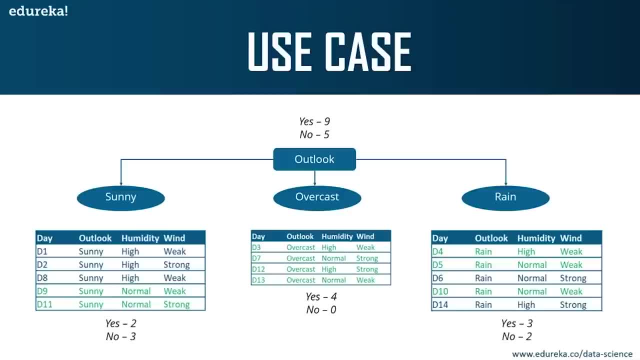 In the data set, It is a hundred percent pure subset, right? So we want variables like these in order to build a model. All right now, we don't always get lucky and we don't always find variables that will result in pure subsets. 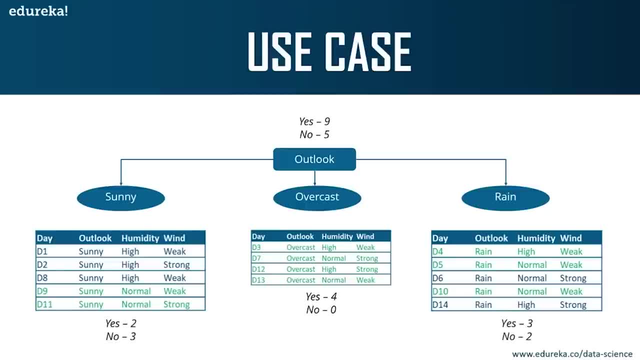 That's why we have the measure entropy. So the lesser the entropy of a particular variable, the most significant that variable will be. So in a decision tree, the root node is assigned the best attribute, so that the decision tree can predict the most precise outcome. meaning that 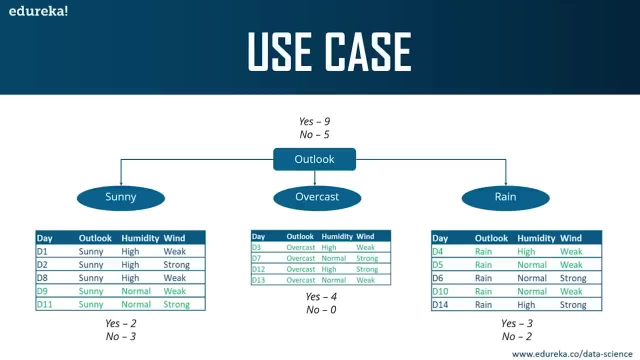 which is sunny, overcast and rain. So, basically, outlook can have three values: Either it can be sunny, it can be overcast or it can be rainy. Okay, Now these three values are assigned to the immediate branch nodes and for each of these values, 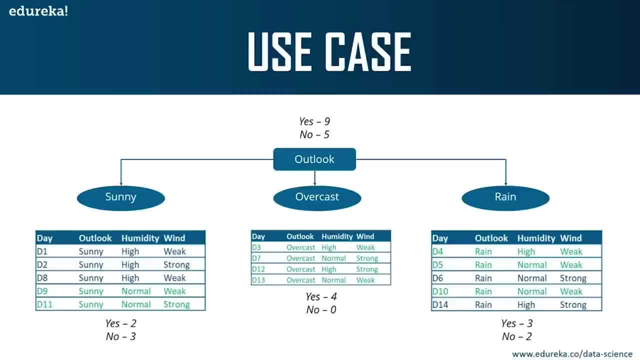 the possibility of play is equal to yes is calculated, So the sunny and the rain branches will give you an impure output, meaning that there is a mix of yes and no right. There are two yeses here, three nos here. There are three yeses here and two nos over here. 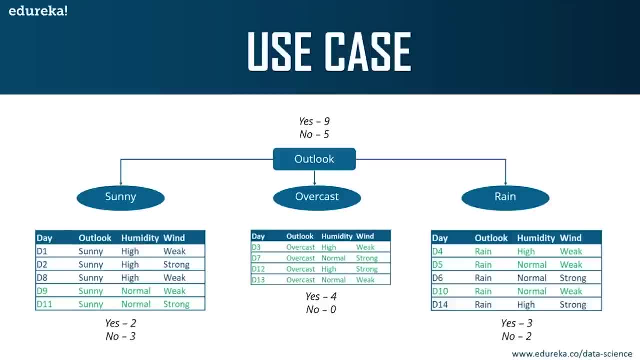 But when it comes to the overcast variable, it results in a hundred percent pure subset. All right, This shows that the overcast variable will result in a definite and certain output. This is exactly what entropy is used to measure. All right. 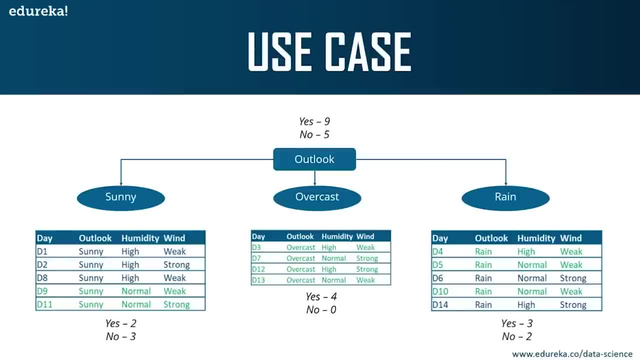 It calculates the impurity or the uncertainty, All right. So the lesser the uncertainty or the entropy of a variable, more significant is that variable. So when it comes to overcast, there's literally no impurity in the data set. It is a hundred percent pure subset. 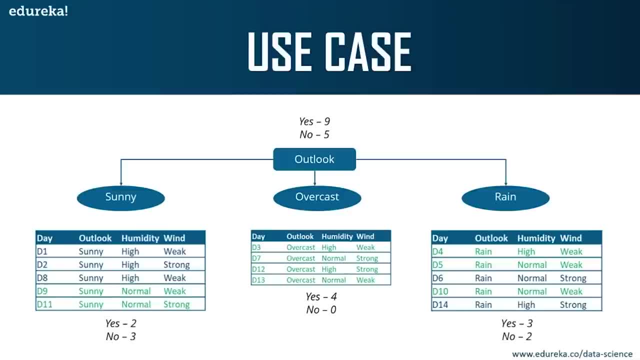 right. So we want variables like these in order to build a model. All right. Now, we don't always get lucky and we don't always find variables that will result in pure subsets. That's why we have the measure entropy, So the lesser the entropy of a particular variable. 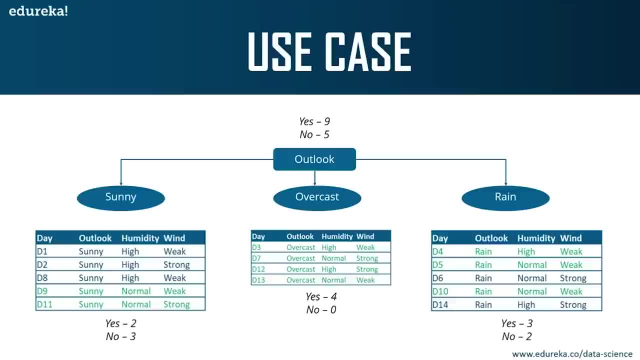 the most significant that variable will be. So in a decision tree, the root node is assigned the best attribute, so that the decision tree is assigned the best attribute. Decision tree can predict the most precise outcome, meaning that on the root node you should have the most significant variable. 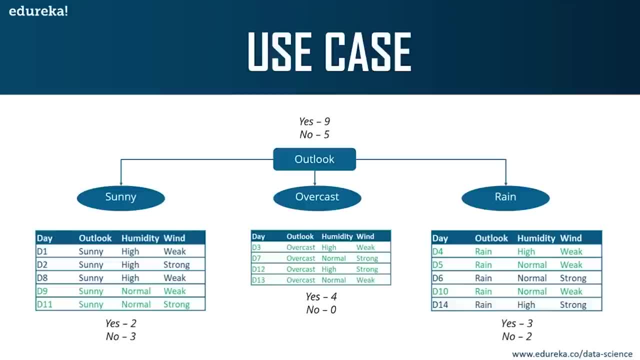 All right, That's why we've chosen outlook. All right. Now some of you might ask me: why haven't you chosen overcast? Now, guys, overcast is not a variable. It is a value of the outlook variable. All right. 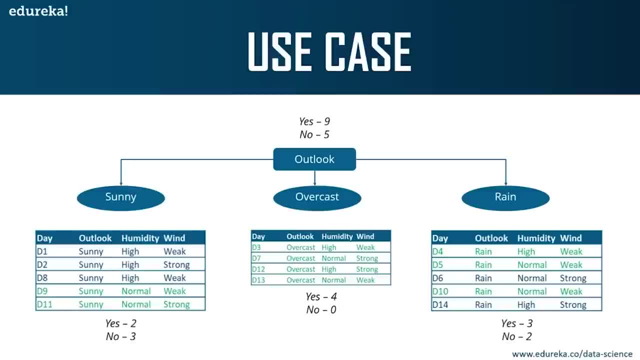 That's why we've chosen outlook here, because it has a hundred percent pure subset, which is overcast. All right. Now the question in your head is: how do I decide, Decide which variable or attribute best splits the data? Now, right now. 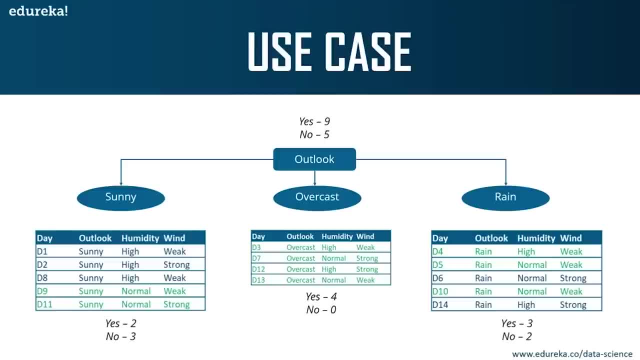 on the root node, you should have the most significant variable. All right, That's why we've chosen Outlook, All right. Now some of you might ask me: why haven't you chosen overcast? now, guys, overcast is not a variable, It is a value of the Outlook variable. 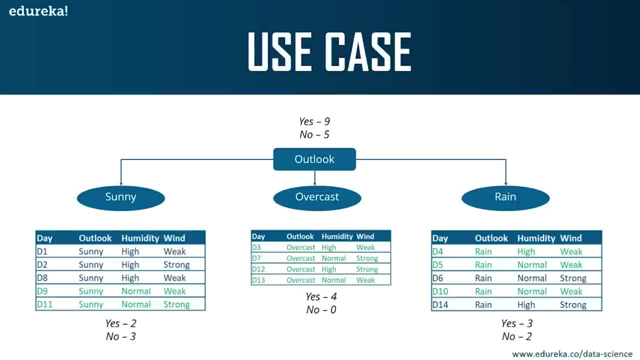 All right, that's why we've chosen Outlook here, because it has a hundred percent pure subset, which is overcast. All right. Now the question in your head is: how do I decide which variable or attribute best splits the data? Now, right now, I know I looked at the data and I told you that you 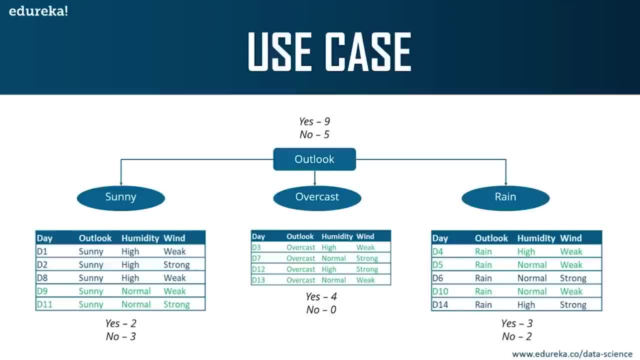 know, here we have a hundred percent pure subset. but what if it's a more complex problem and you're not able to understand which variable will best split the data? So, guys, when it comes to decision trees, information and gain and entropy will help you understand which variable will best split the. 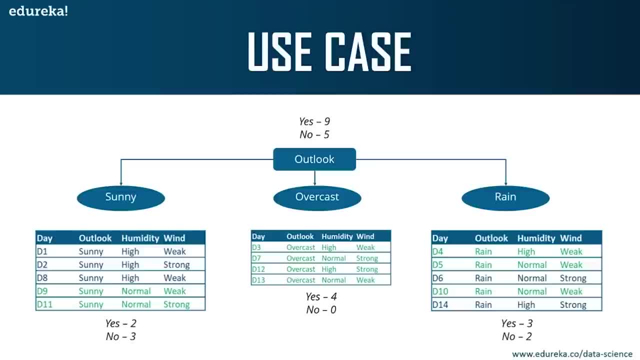 data set, All right, or which variable you have to assign to the root node, because whichever variable is assigned to the root node, it will best split the data set And it has to be the most significant variable, All right. So how we can do this is we need to use information gain and entropy. 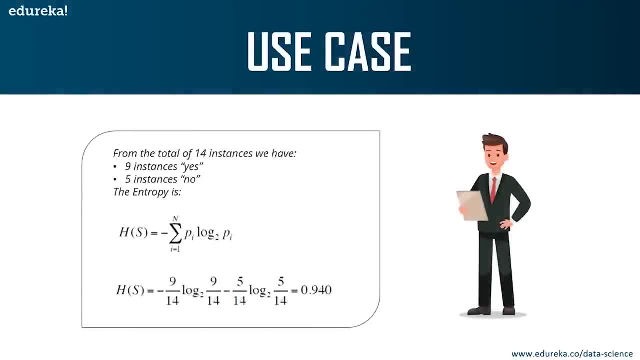 So from the total of the 14 instances that we saw, nine of them said yes and five of the instances said no, that you cannot play on that particular day, All right, So how do you calculate the entropy? So this is the formula. You just substitute the values in the formula. 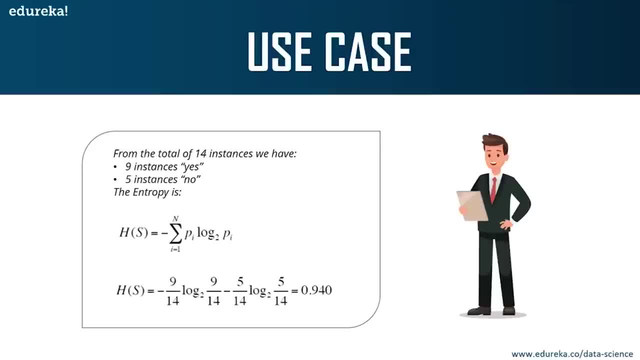 So when you substitute the values in the formula, you'll get a value of 0.9 for 0.. All right, This is the entropy, or this is the uncertainty of the data present in our sample. Now, in order to ensure that we choose the best variable for the root, 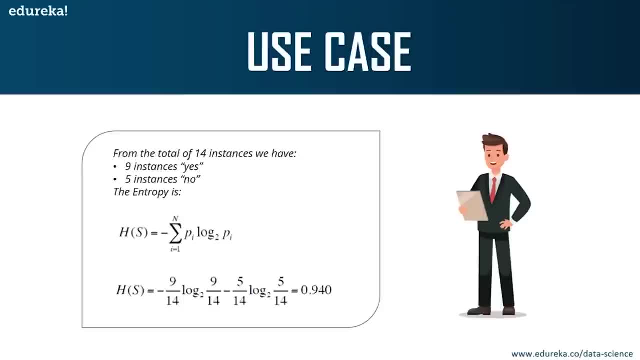 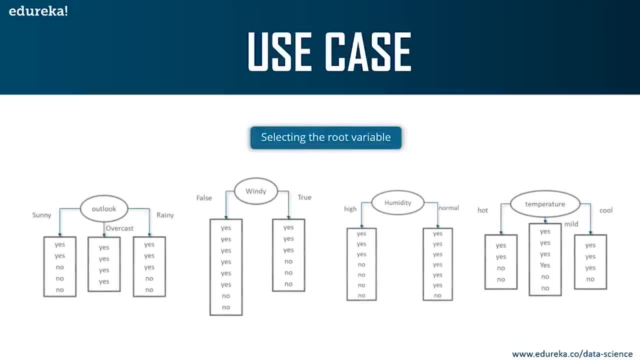 node. Let us look at all the possible combinations that you can use on the root node. Okay, so these are all the possible combinations. You can either have Outlook, you can have windy, humidity or temperature. Okay, these are our four variables, and you can have any one of these. 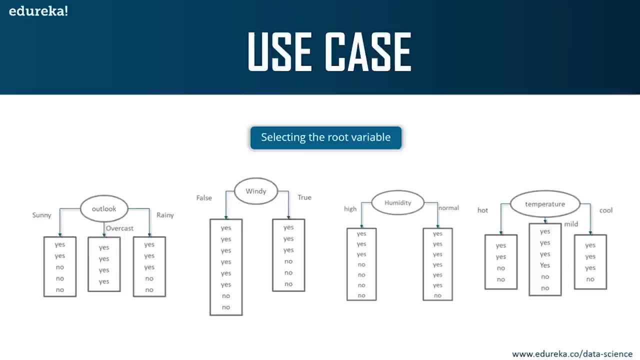 variables as your root node, but how do you select which variable best fits the root node? That's what we are going to see: by using information gain and entropy. So, guys, now the task at hand is to find the information gain for each of these attributes. 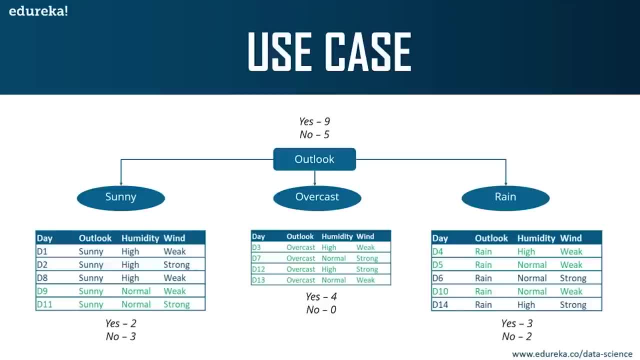 I know. I looked at the data and I told you that you know, here we have a hundred percent pure subset. but what if it's a more complex problem and you're not able to understand which variable will best split the data? So, guys, 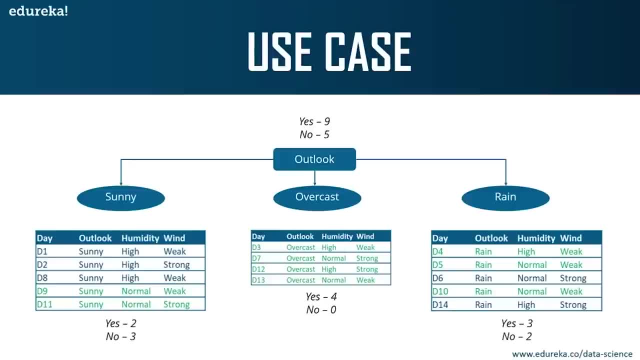 when it comes to decision trees, information and gain and entropy will help you understand which variable will best split the data set- All right- or which variable you have to assign to the root node, because whichever variable is assigned to the root node, it will best split the data set and it has to be the most significant variable. 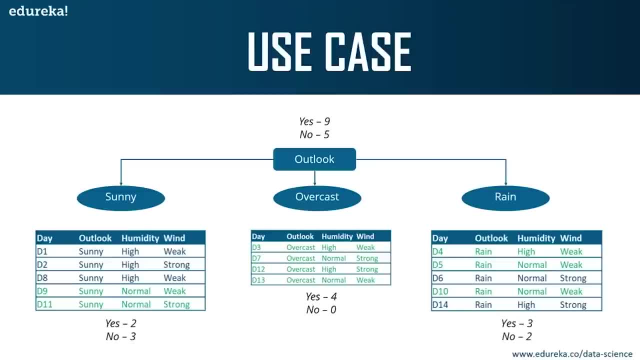 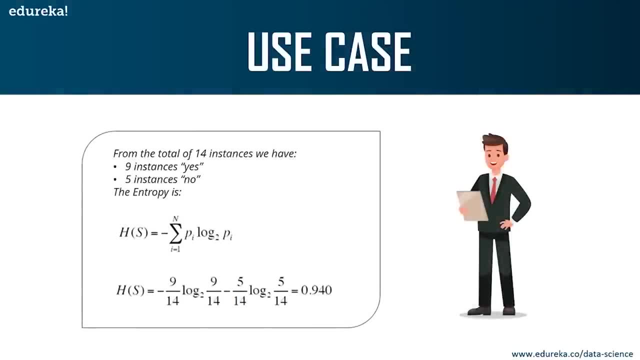 All right. So how we can do this is we need to use information gain and entropy. So from the total of the 14 instances that we saw, nine of them said yes and five of the instances said no, that you cannot play on that particular day. 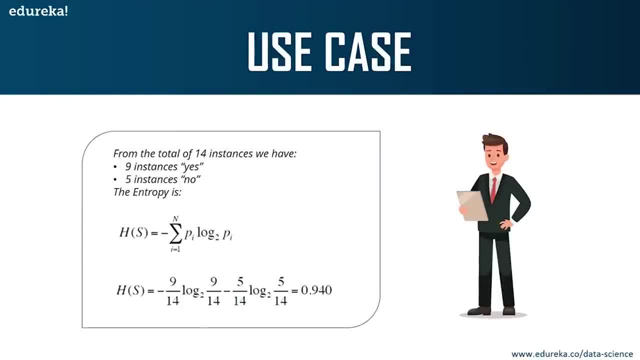 All right. So how do you calculate the entropy? So this is the formula: You just substitute the values in the formula. So when you substitute the values in the formula, you'll get a value of 0.940.. All right. 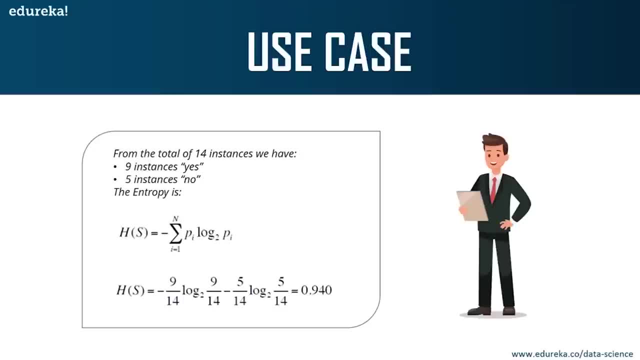 This is the entropy, or this is the uncertainty, of the data present in our sample. Now, in order to ensure that we choose the best variable for the root node, Let us look at all the possible combinations that you can use on the root node. Okay, 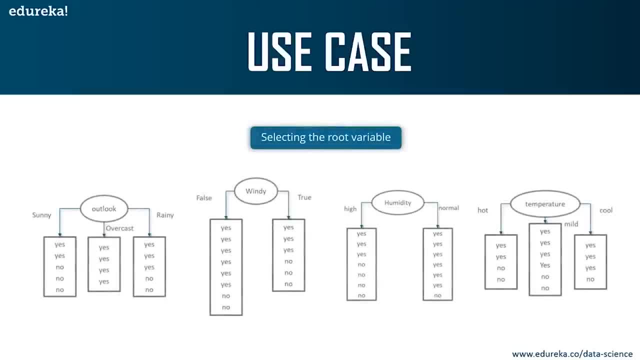 So these are all the possible combinations. You can either have Outlook, you can have windy, humidity or temperature. Okay, These are our four variables, and you can have any one of these variables as your root. But how do you select which variable best fits the root node? 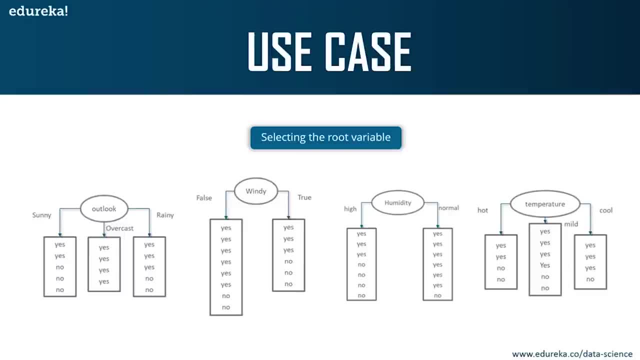 That's what we are going to see by using information gain and entropy. So, guys, now the task at hand is to find the information gain for each of these attributes. All right, So for Outlook, for windy, for humidity and for temperature, we're going to find out the information gain. 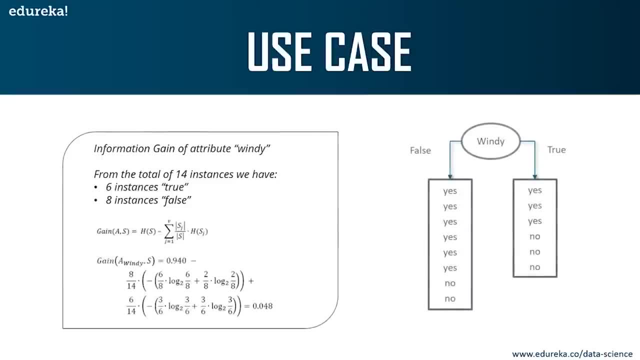 All right. Now a point to remember is that the variable that results in the highest information gain must be chosen because it will give us the most precise and output information. All right, So the information gain for attribute windy will calculate that first. here We have six instances of true and eight instances of false. 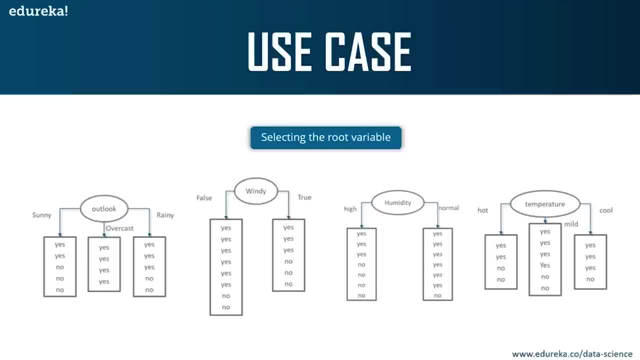 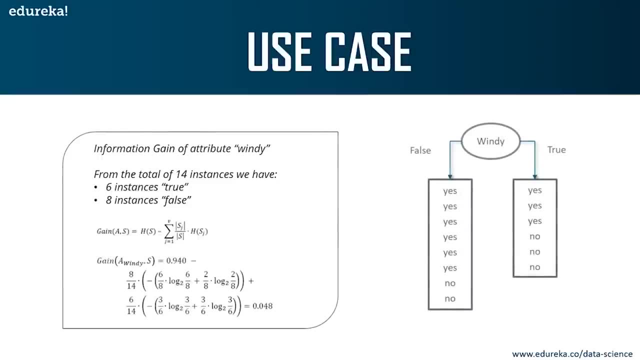 All right. So for Outlook for windy, for humidity and for temperature, we're going to find out the information gain All right now. a point to remember is that the variable that results in the highest information gain must be chosen because it will give us the most. 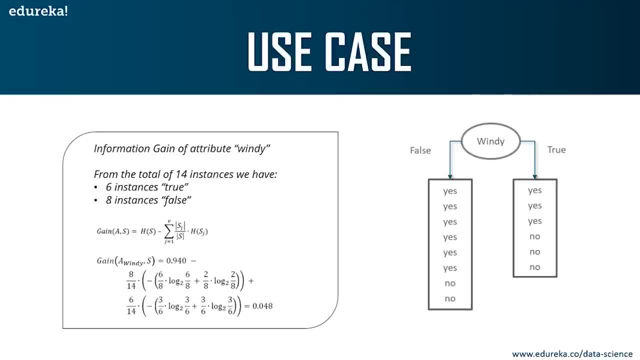 precise and output information. All right. so the information gain for Attribute windy will calculate that first. here We have six instances of true and eight instances of false. Okay, so when you substitute all the values in the formula you'll get a. 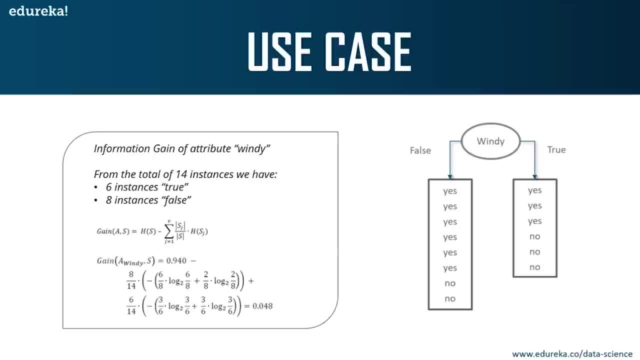 value of 0.048.. So we get a value of 0.048.. Now, this is a very low value for information gain. All right, so the information that you're going to get from windy attribute is pretty low. So let's calculate the information gain of attribute. 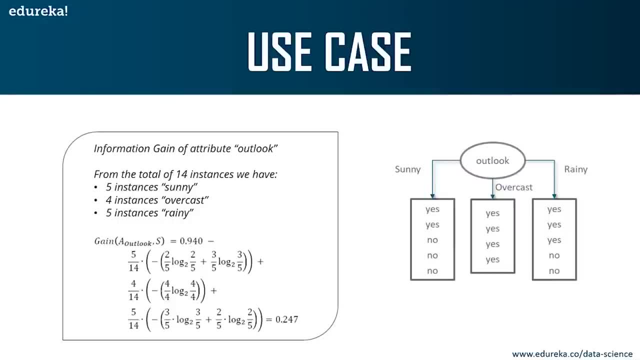 Outlook: All right. So from the total of 14 instances, we have five instances which say sunny, four instances which are overcast and five instances which are rainy. All right for sunny, We have three yeses and two knowns for overcast. 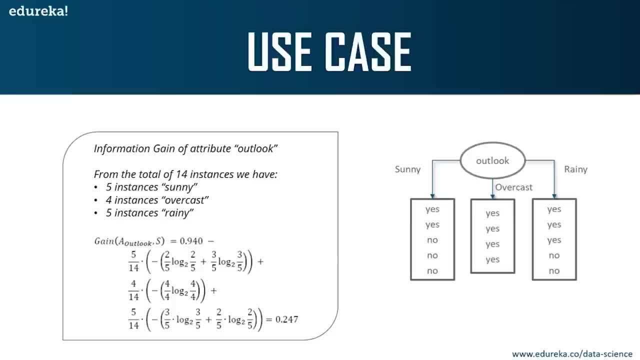 We have all the four as yes for rainy. We have three yes and two knowns. Okay, So when you calculate, the information gain of the Outlook variable will get a value of 0.247. now compare this to the information gain of the windy. 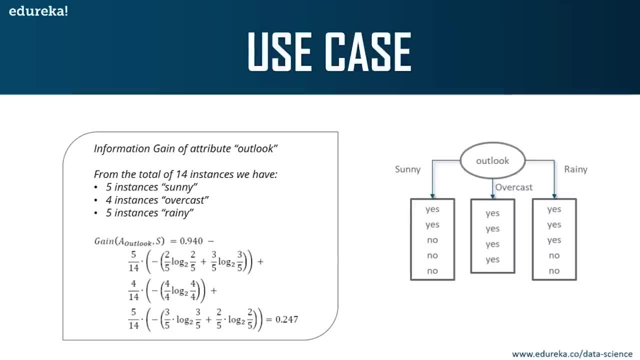 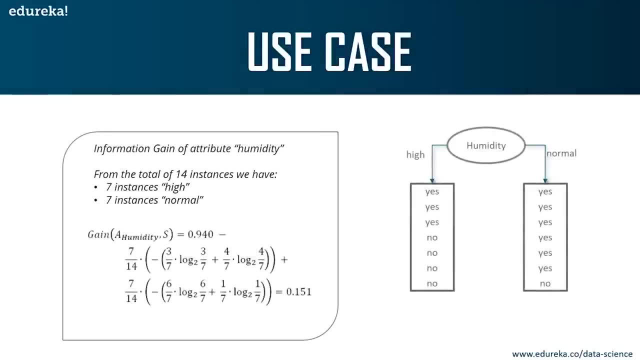 Attribute. This value is actually pretty good, right? We have 0.247, which is a pretty good value for information gain. Now let's look at the information gain of attribute humidity. Now, over here We have seven instances with say high and seven instances with say normal. 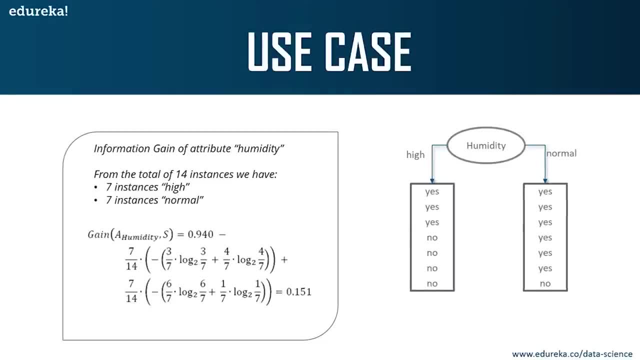 right and under the high branch node We have three instances with say yes and the rest four instances with say no. similarly, under the normal branch, We have one, two, three, four, five, six, seven instances Which say yes and one instance which says no. 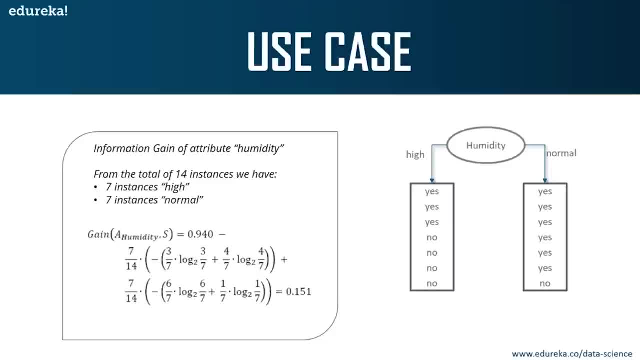 All right. So when you calculate the information gain for the humidity variable, you're going to get a value of 0.151.. Now, this is also a pretty decent value, But when you compare it to the information gain of the attribute Outlook, it is less. right now. 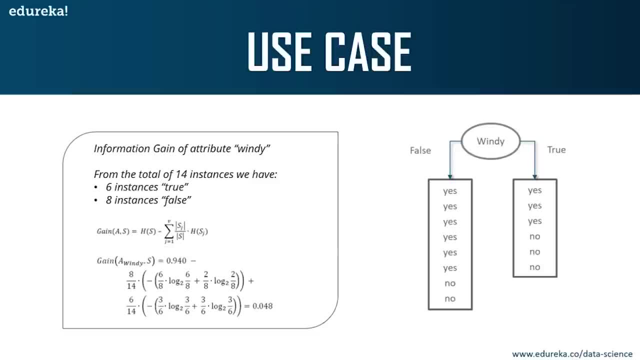 Okay, So when you substitute all the values in the formula, you'll get a value of 0.048.. So we get a value of 0.048.. Now, this is a very low value for information gain. All right, So the information that you're going to get from windy attribute is pretty low. 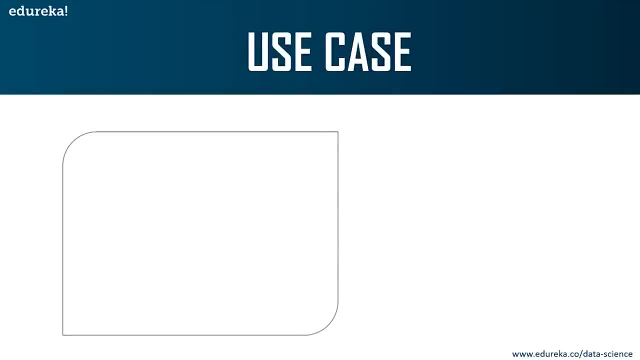 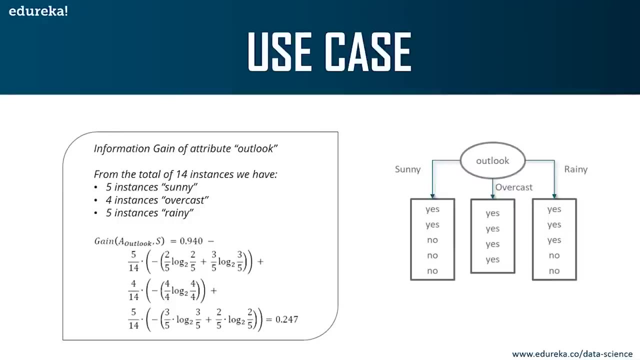 So let's calculate the information gain of attribute Outlook. All right, So from the total of 14 instances, we have five instances which say sunny, for instances which are overcast and five instances which are rainy. All right for sunny. 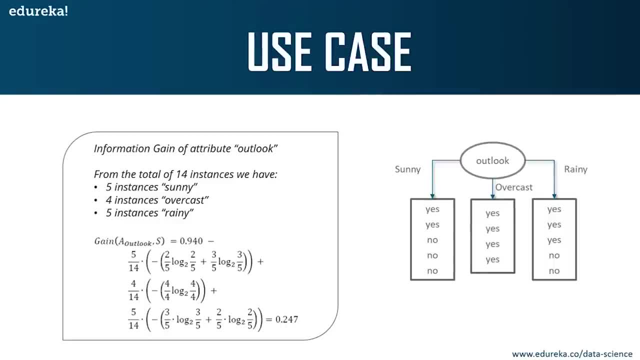 We have three yeses and two knowns. for overcast, We have all the four. as yes. for rainy, We have three yes and two knowns. Okay, So when you calculate the information gain of the Outlook variable, we'll get a value of 0.048.. 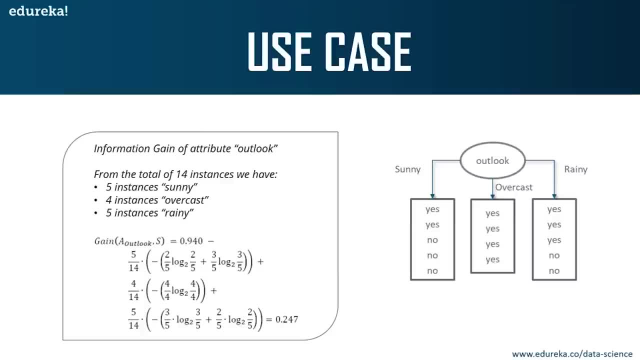 Now compare this to the information gain of the windy attribute. This value is actually pretty good, right? We have 0.247, which is a pretty good value for information gain. Now let's look at the information gain of attribute humidity. 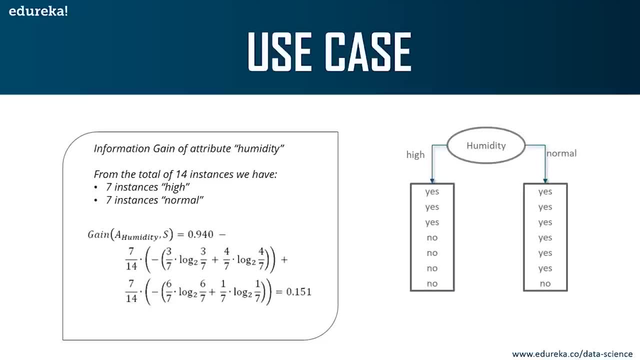 Now over here we have seven instances which say high and seven instances which say normal, right And under the high branch node we have three instances which say yes and the rest four instances which say no. Similarly, under the normal branch. 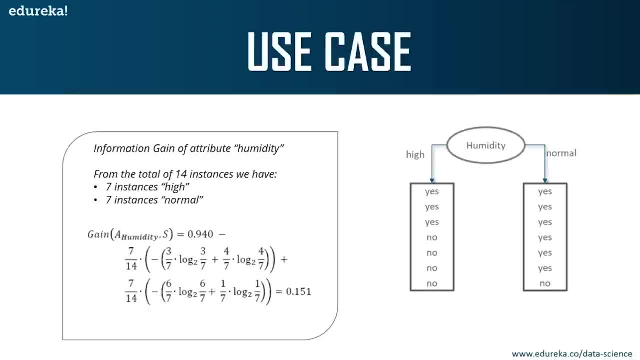 we have one, two, three, four, five, six, seven instances which say yes and one instance which says no. All right, So when you calculate the information gain for the humidity variable, you're going to get a value of 0.151.. 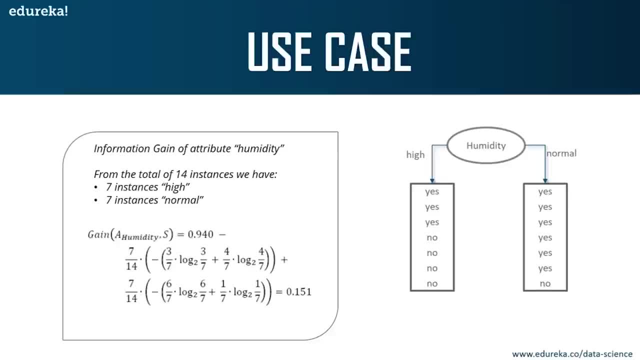 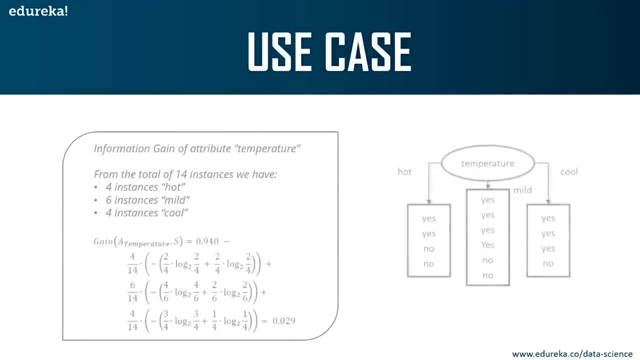 Now, this is also a pretty decent value, But when you compare it to the information gain of the attribute Outlook, it is less right. Now let's look at the information gain of attribute temperature. All right, So the temperature can hold repeat. 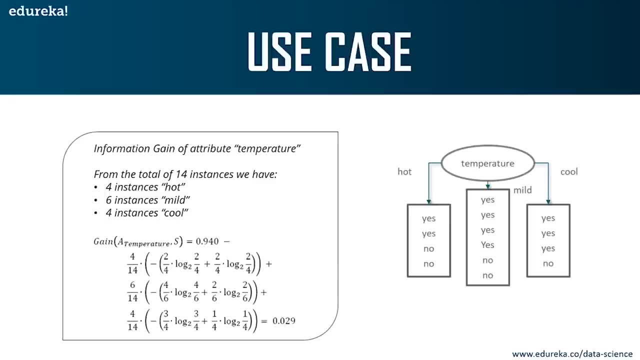 So basically the temperature attribute can hold hot, mild and cool. Okay, under hot, we have two instances which says yes and two instances for no. Under mild, we have four instances of yes and two instances of no, And under cool, 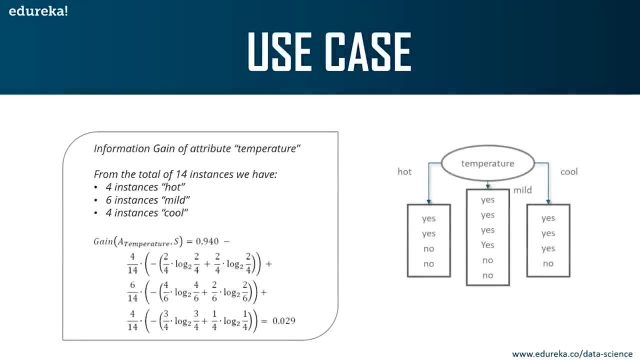 Let's look at the information gain of attribute temperature. All right, So the temperature can hold repeat. So basically, the temperature attribute can hold hot, mild And cool. okay under hot, We have two instances which says yes and two instances for no under mild. 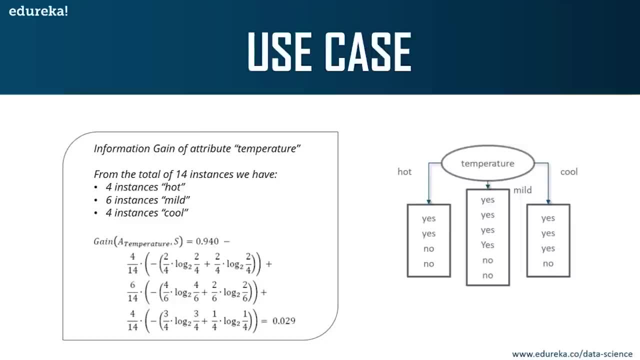 We have four instances of yes and two instances of no, and under cool, We have three instances of yes and one instance of no. All right Now, when you calculate the information gain for this attribute, you'll get a value of 0.029, which is again very less. 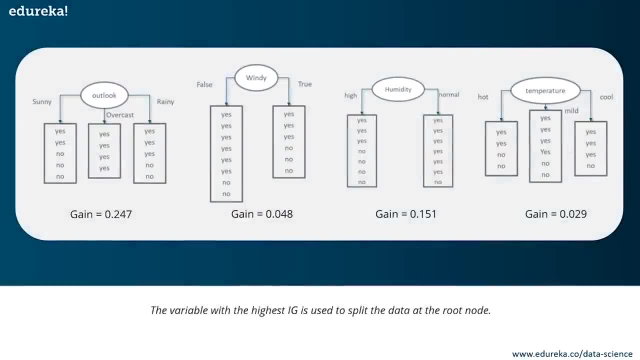 So what you can summarize from here is, if we look at the information gain for each of these variable, We'll see that, for Outlook, We have the maximum gain. All right, We have 0.247, which is the highest information gain value, and you must. 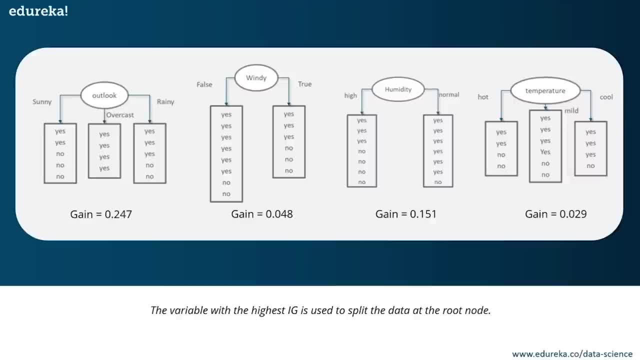 always choose a variable with the highest information gain to split the data at the root node. So that's why we assign the Outlook variable at the root node. All right, So, guys, I hope this use case was clear. If any of you have doubts, please keep commenting those doubts. 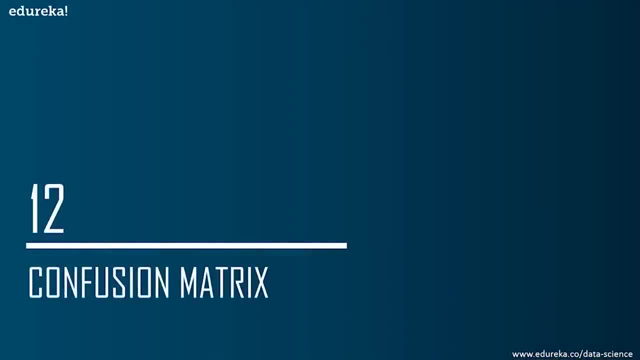 Now let's move on and look at what exactly a confusion matrix is. Now, the confusion matrix is the last topic for descriptive statistics. All right, After this, I'll be running a short demo where I'll be showing you how you can calculate mean, median mode and standard deviation variance. 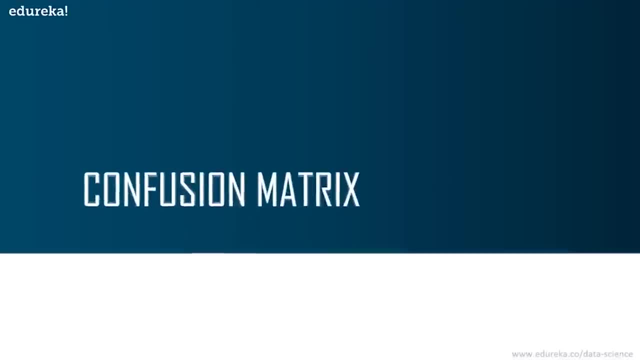 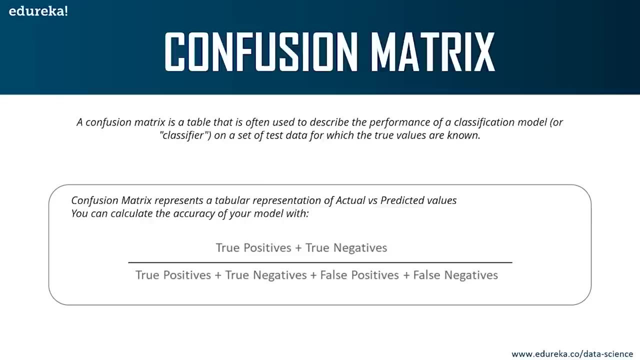 and all of those values by using R. Okay, So let's talk about confusion matrix. Now, guys, what is a confusion matrix? Now, don't get confused. This is not any complex topic. Now, confusion matrix is a matrix that is often used to describe the 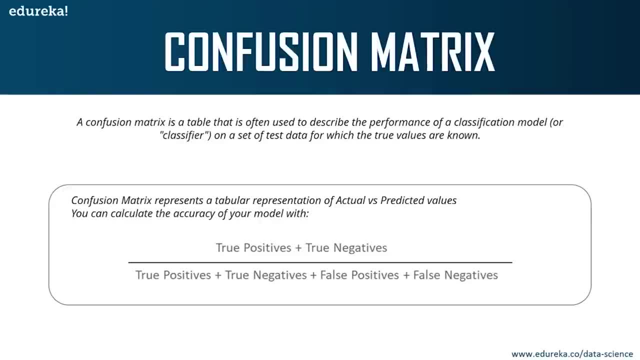 performance of a model, All right, And this is specifically used for classification models or a classifier, And what it does is it will calculate the accuracy or it will calculate the performance of your classifier by comparing your actual results and your predicted results. All right. 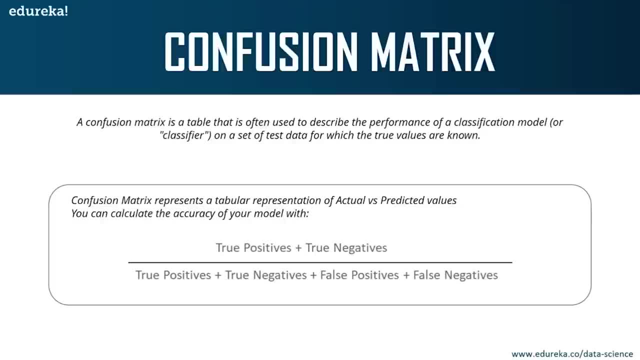 So this is what it looks like: True positive, true negative and all of that. Now, this is a little confusing. I'll get back to what exactly true positive, true negative and all of this stands for. For now, let's look at an example and let's try and understand what 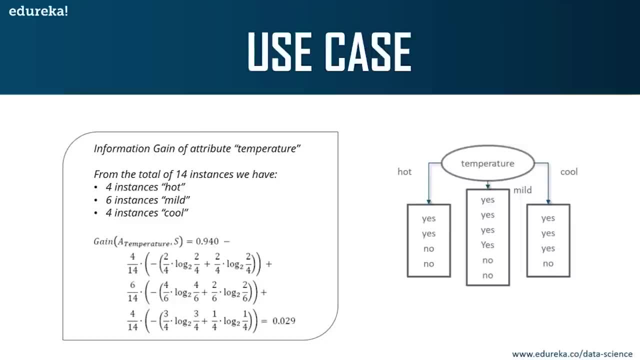 we have three instances of yes and one instance of no. All right Now, when you calculate the information gain for this attribute, you'll get a value of 0.029, which is again very less. So what you can summarize from here is: 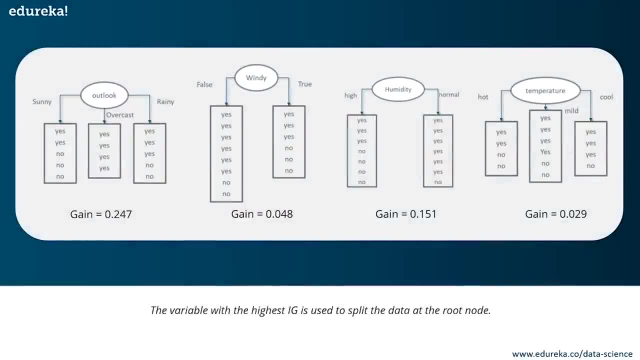 if we look at the information gain for each of these variables, we'll see that for Outlook, we have the maximum gain. All right, we have 0.247, which is the highest information gain value, And you must always choose a variable with the highest information. 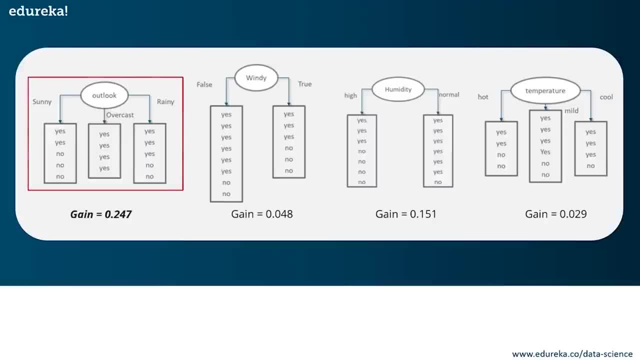 gain to split the data at the root node. So that's why we assign the Outlook variable at the root node. All right, So, guys, I hope this use case was clear. If any of you have doubts, please keep commenting those doubts. 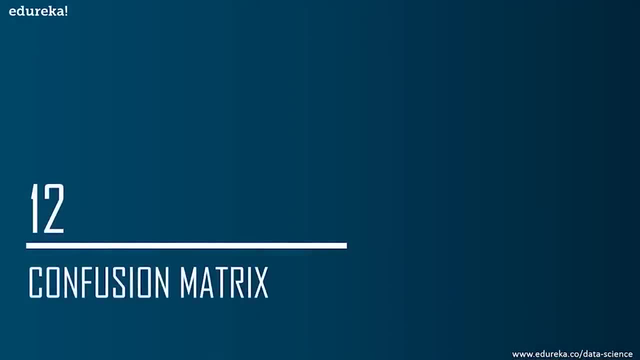 Now let's move on and look at what exactly a confusion matrix is. Now the confusion matrix is the last topic for descriptive statistics. All right, After this, I'll be running a short demo where I'll be showing you how you can calculate. 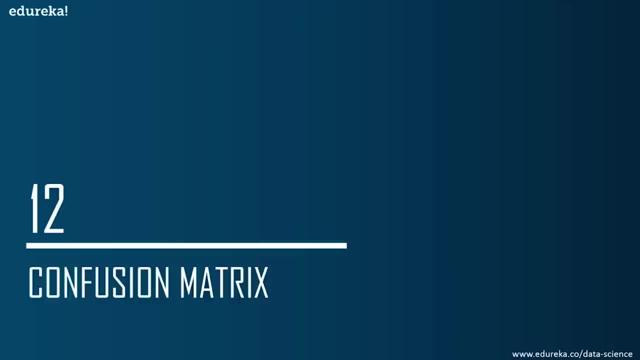 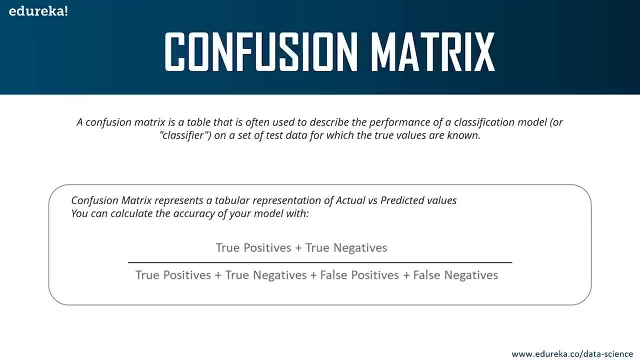 mean median mode and standard deviation, variance, and all of those values by using R. Okay, So let's talk about confusion matrix. Now, guys, what is a confusion matrix? Now, don't get confused, This is not. 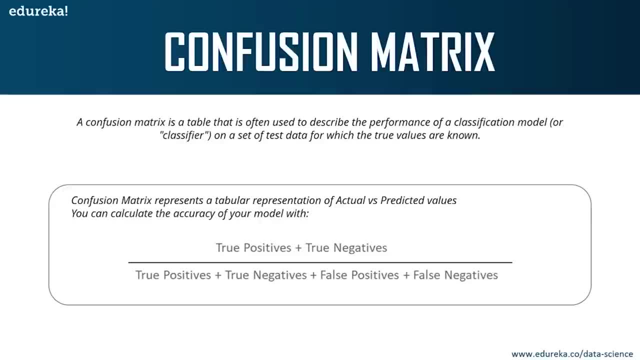 any complex topic. Now a confusion: matrix is a matrix that is often used to describe the performance of a model. All right, and this is specifically used for classification models, or a classifier, And what it does is it will calculate the accuracy or it will. 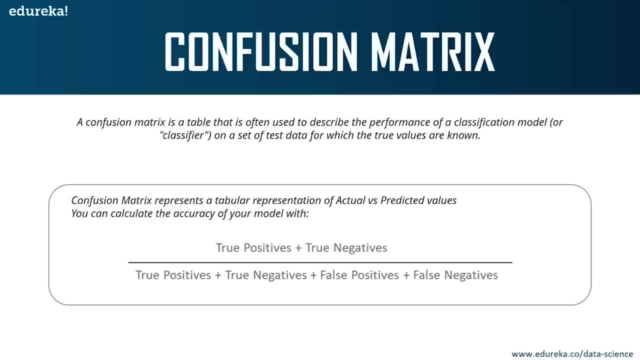 calculate the performance of your classifier by comparing your actual results and your predicted results. All right, So this is what it looks like: Two positive plus two negative and all of that. Now, this is a little confusing. I'll get back to what exactly true positive. 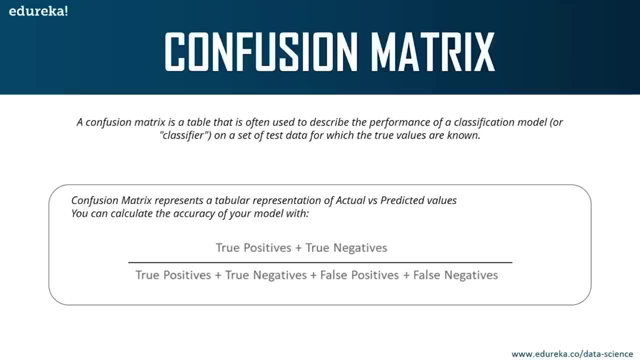 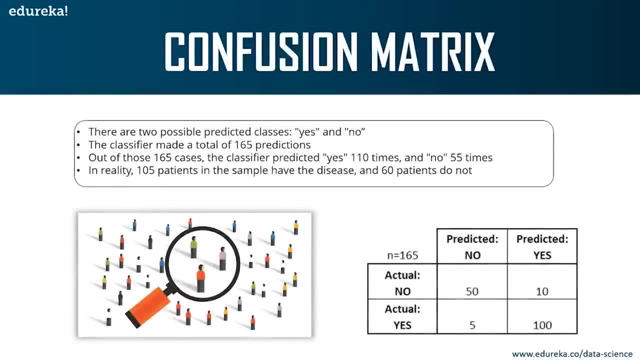 true, negative and all of this stands for. For now, let's look at an example and let's try and understand what exactly confusion matrix is. So, guys, I made sure that I put examples after each and every topic because it's important you understand the practical part of statistics. 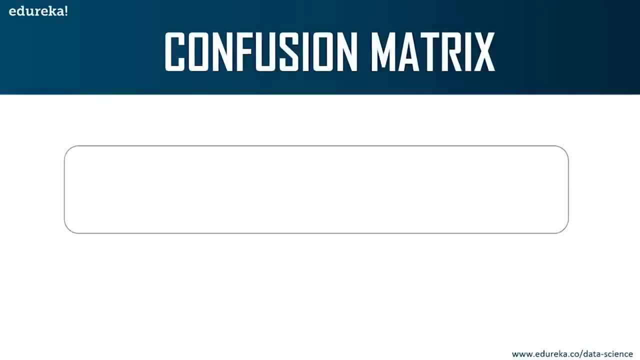 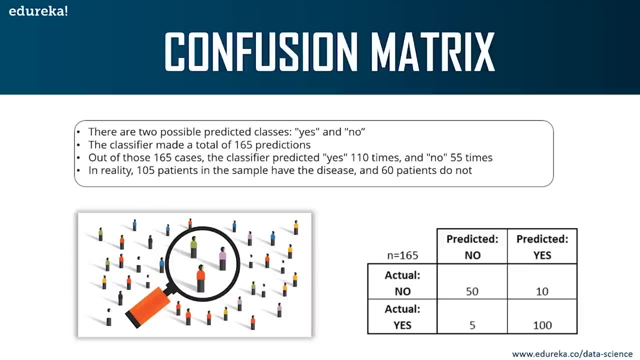 exactly confusion matrix is. So, guys, I made sure that I put examples after each and every topic because it's important you understand the practical part of statistics. All right, Statistics has literally nothing to do with theory. You need to understand how calculations are done in statistics. 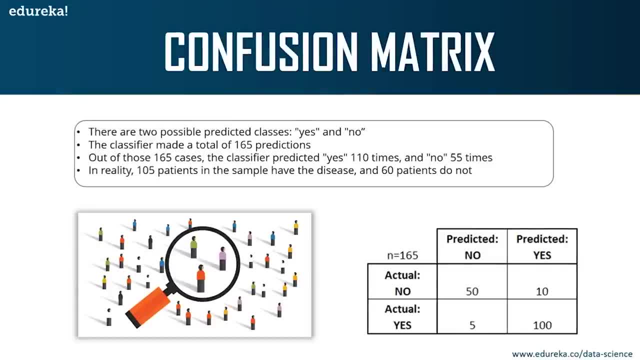 Okay, So here, what I've done is now let's look at a small use case. Okay, Let's consider that you're given data about 165 patients, out of which 105 patients have a disease and the remaining 50 patients don't. 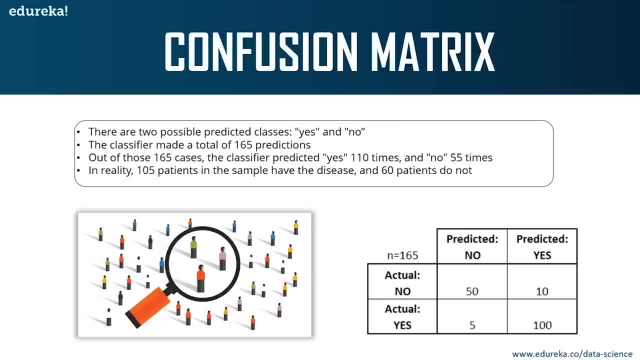 have a disease. Okay, So what you're going to do is you'll build a classifier that predicts by using these 165 observations. You'll feed all of these 165 observations to your classifier and it will predict the output every time a new patient's detail is fed to the 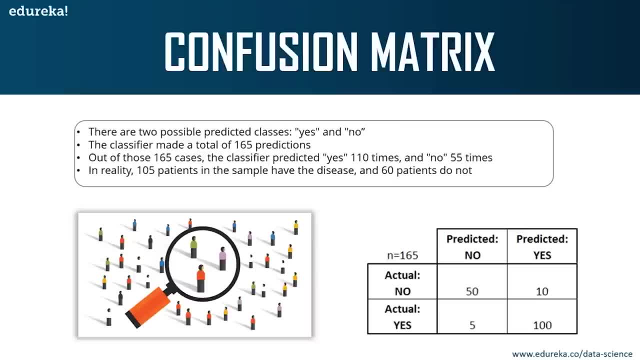 classifier Right Now. out of these 165 cases, let's say that the classifier predicted yes 110 times And no 55 times. All right, So yes basically stands for yes- the person has a disease, and no stands for no- the person does not have a disease. 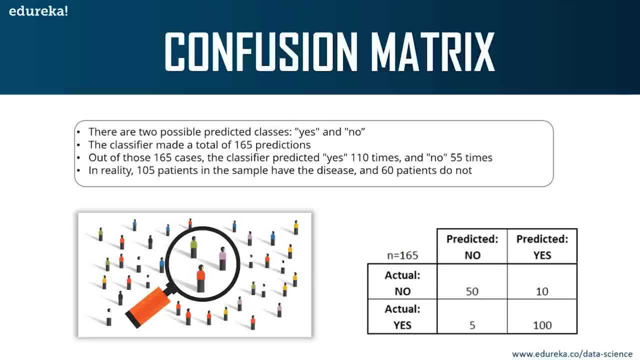 All right, That's pretty self-explanatory, But yeah, so it predicted that 110 times patient has a disease and 55 times that, no, the patient doesn't have a disease. However, in reality, only 105 patients in the sample have the disease and. 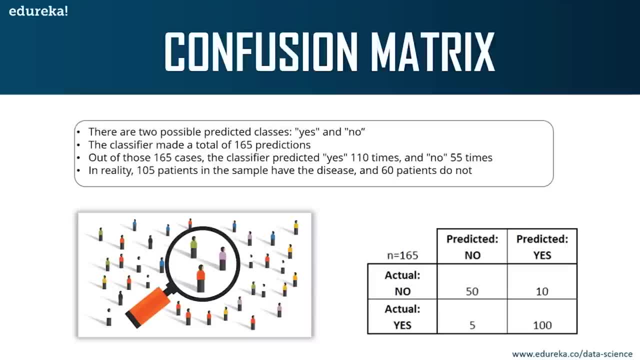 60 patients who do not have the disease Right. So how do you calculate the accuracy of your model? You basically build the confusion matrix, All right. this is how the matrix looks like and basically denotes the total number of observations that you have, which is 165 in our case. 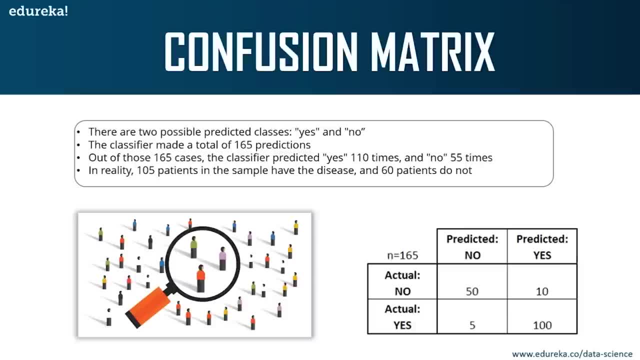 actual denotes the actual values in the data set and predicted denotes the predicted values by the classifier. So the actual value is no here and the predicted value is no here. So your classifier was correctly able to classify 50 cases As no. all right, since both of these are no, so 50 it was correctly able. 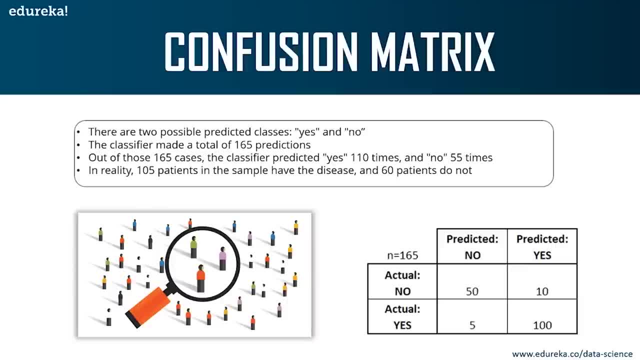 All right, statistics has literally nothing to do with theory. You need to understand how calculations are done in statistics. Okay, So here, what I've done is now let's look at a a small use case. Okay, Let's consider that you're given data about hundred and sixty-five. 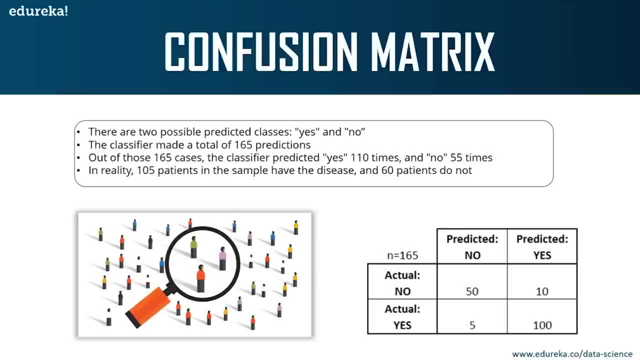 patients, out of which hundred and five patients have a disease and the remaining 50 patients don't have a disease. Okay, So what you're going to do is you will build a classifier that predicts by using these hundred and sixty-five observations. You'll feed all of these 165 observations to your classifier and 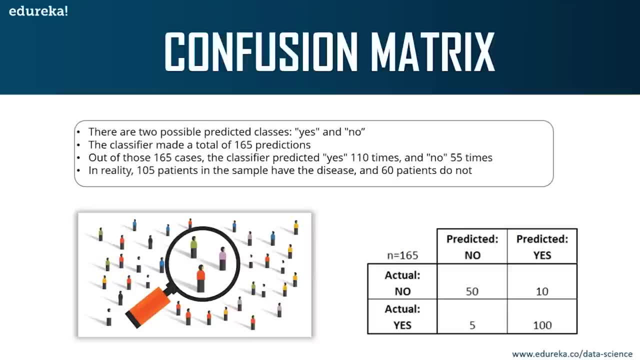 it will predict the output every time a new patient's detail is fed to the classifier. right Now, out of these 165 cases, let's say that the classifier predicted Yes 110 times and no 55 times. All right, So yes. 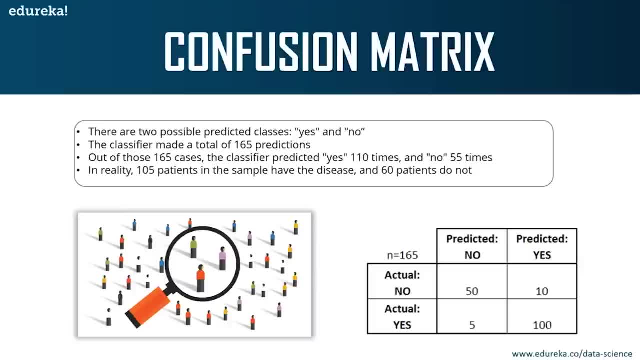 basically stands for yes, the person has a disease, and no stands for no, the person does not have a disease. All right, that's pretty self-explanatory, But yeah, so it predicted that 110 times patient has a disease and 55 times that no. 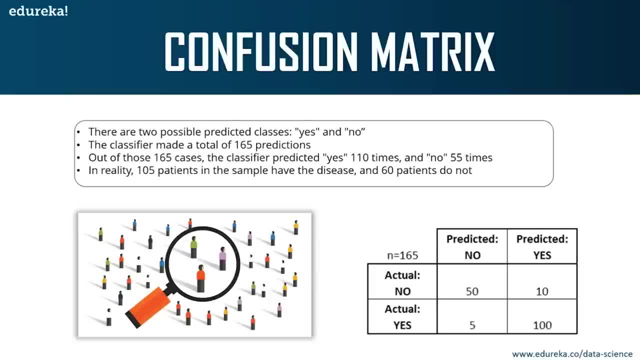 the patient doesn't have a disease. However, in reality, only hundred and five patients in the sample have the disease and 60 patients who do not have the disease right. So how do you calculate the accuracy of your model? You basically build the confusion Matrix. 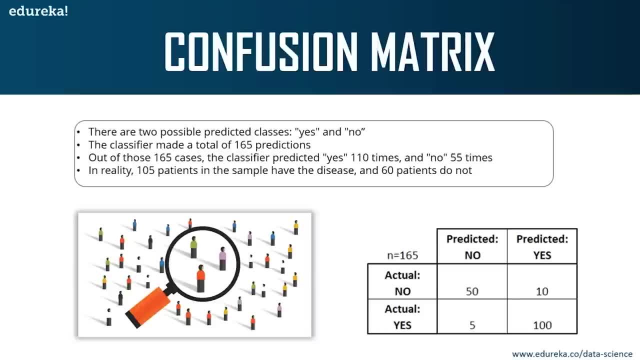 All right, this is how the Matrix looks like and basically denotes the total number of observations that you have, which is 165 in our case. actual denotes the actual values in the data set and predicted denotes the predicted values by the classifier. So the actual value is no here and the predicted value is no here. 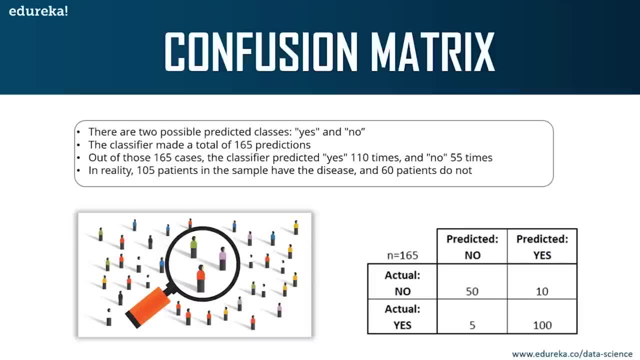 So your classifier was correctly able to classify 50 cases as no. All right, since both of these are no, so 50 it was correctly able to classify, but 10 of these cases it incorrectly classified, meaning that your actual value here is no. 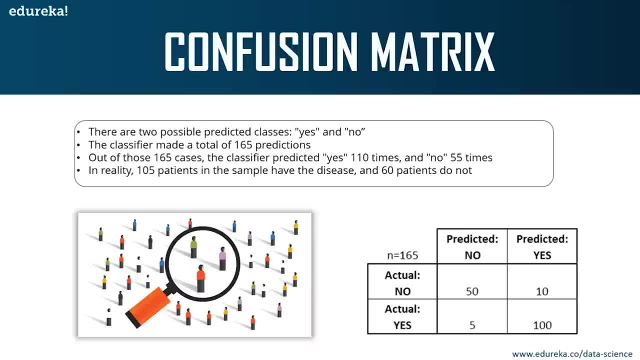 but your classifier predicted it as yes, All right, that's why this 10 over here. Similarly, it wrongly predicted that five patients do not have diseases, Whereas they actually did have diseases, and it correctly predicted hundred patients which have the disease. All right. 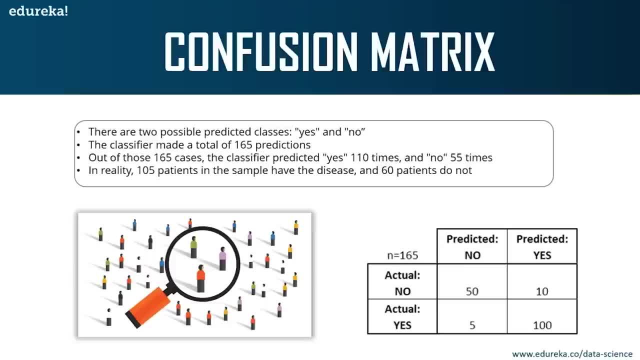 to classify but 10 of these cases. it incorrectly classified, meaning that your actual value here is no, but your classifier predicted it as yes. All right, That's why this 10 over here. Similarly, it wrongly predicted that five patients do not have diseases. 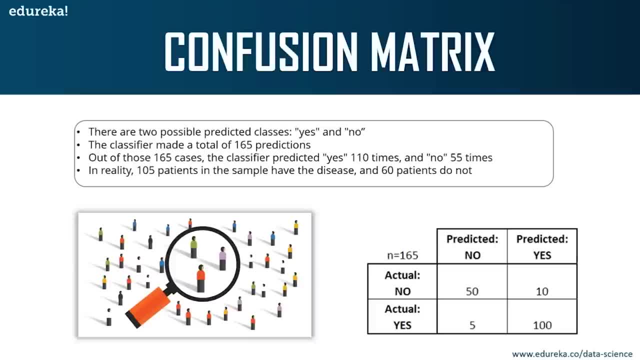 whereas they actually did have diseases, and it correctly predicted hundred patients which have the disease. All right, I know this is a little bit confusing, But if you look at these values, no, no, 50, meaning that it correctly predicted 50 values. 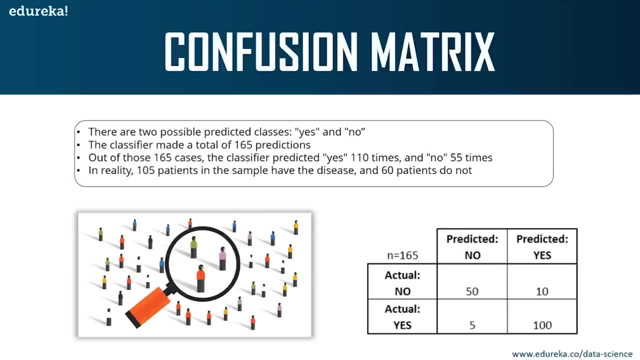 No. Yes means that it wrongly predicted Yes for the values that it was supposed to predict. No, All right. Now, what exactly is this? true positive, true negative and all of that. I'll tell you what exactly it is So true. positive are the cases in which we predicted a yes and they do not. 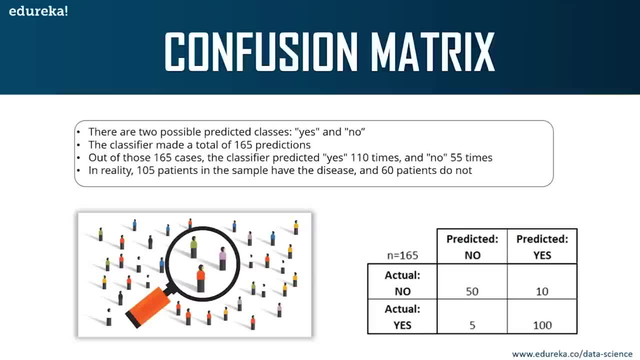 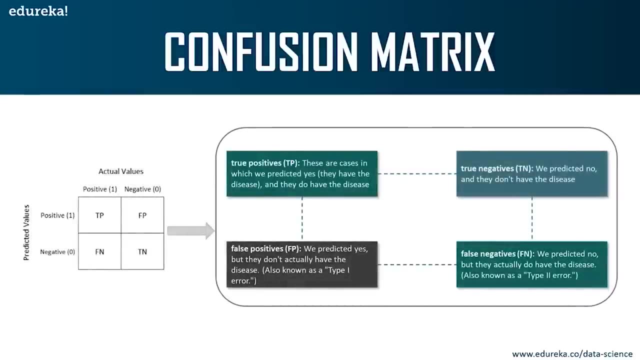 actually have the disease. All right. So it is basically this value, All right. We predicted a yes here, even though they did not have the disease. So we have 10 true positives, right? Similarly, true negative is: we predicted no and they don't have the disease. 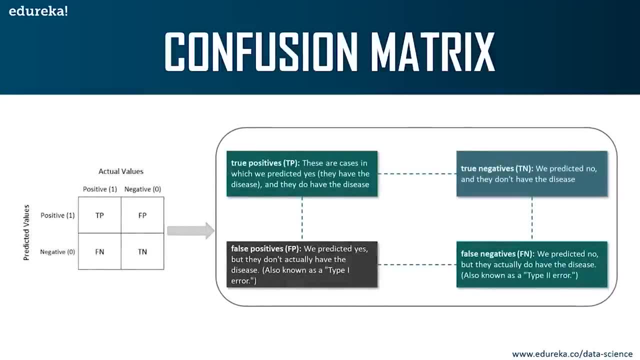 meaning that this is correct. false positive is be predicted Yes, but they do not actually have the disease. All right, This is also known as type 1 error. false negative is we predicted no, but they actually do not have the disease. So, guys, basically false negative and true negatives are basically correct. 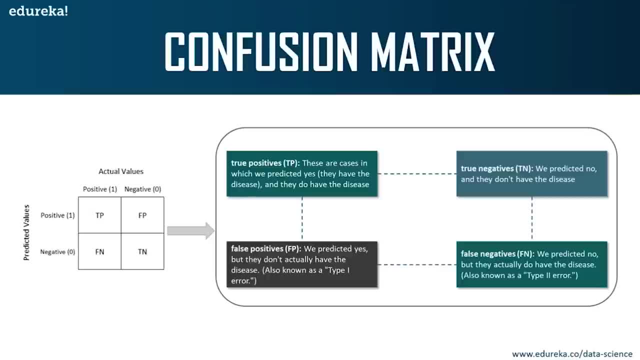 classifications. All right, So this was confusion matrix, and I hope this concept is clear. again, guys, If you have doubts, please comment your doubts in the comment section. So, guys, that was the entire descriptive statistics module, and now we'll discuss about probability. 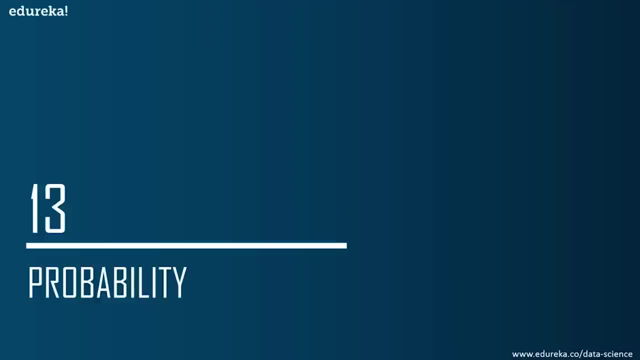 Okay, So before we understand what exactly probability is, let me clear out a very common misconception. people often tend to ask me This question: What is the relationship between statistics and probability? So probability and statistics are related fields, All right, So probability is a mathematical method used for statistical analysis. 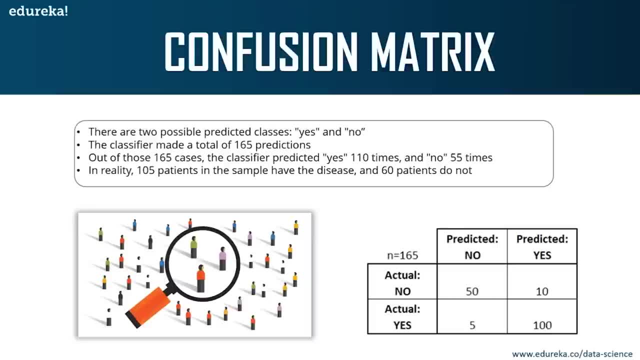 I know this is a little bit confusing, But if you look at these values, no, no, 50, meaning that it correctly predicted 50 values. No, Yes means that it wrongly predicted Yes for the values that it was supposed to predict. 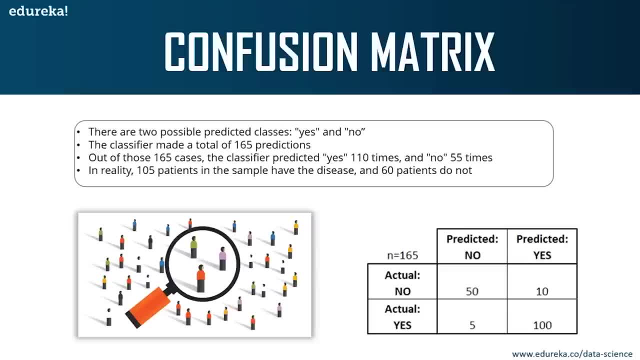 No, All right Now, what exactly is this? true positive, true negative and all of that. I'll tell you what exactly it is So true positive are the cases in which we predicted a yes and they do not actually have the disease. 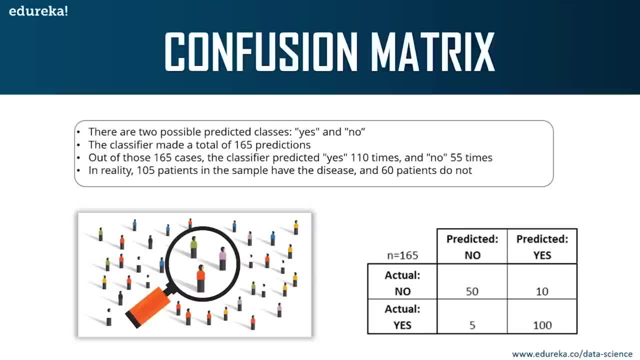 All right. So it is basically this value. All right. We predicted a yes here, even though they did not have the disease. So we have 10 true positives, right. Similarly true negative is we predicted no and they don't have the disease. 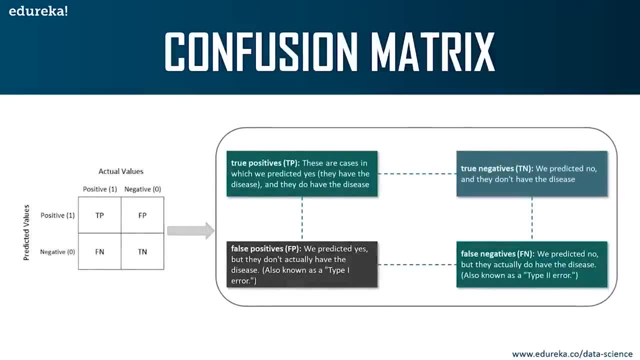 meaning that this is correct. False positive is be predicted: Yes, but they do not actually have the disease. All right, This is also known as type 1 error. False negative is we predicted: no, but they actually do not have the disease. 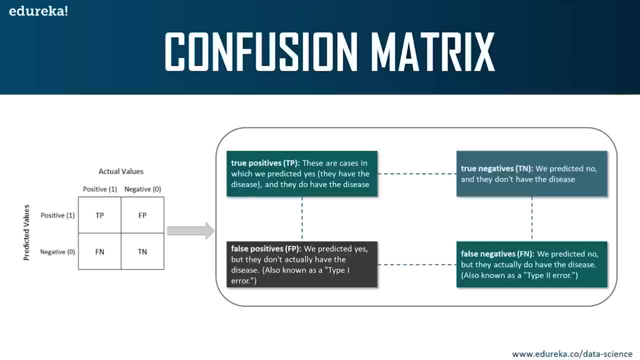 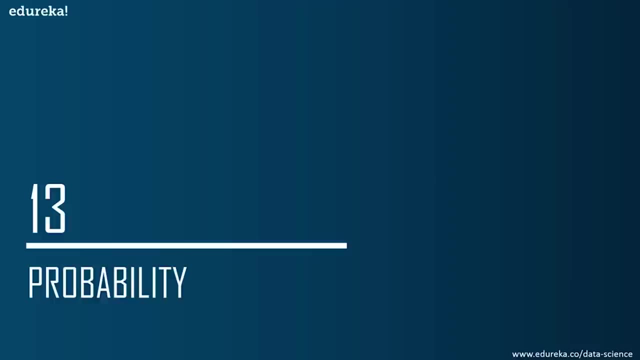 So, guys, basically false negative and true negatives are basically correct classifications, All right, So this was confusion matrix and I hope this concept is clear again. guys, If you have doubts, please comment your doubts in the comment section. So, guys, that was the entire descriptive statistics module. 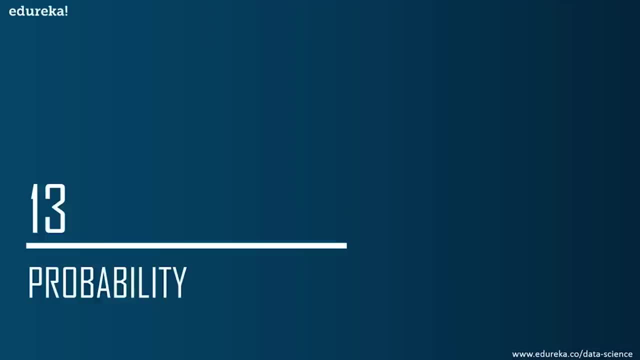 And now we'll discuss about probability. Okay, So before we understand what exactly probability is, let me clear out a very common misconception. People often tend to ask me this question: What is the relationship between statistics and probability? So probability and statistics are related fields. 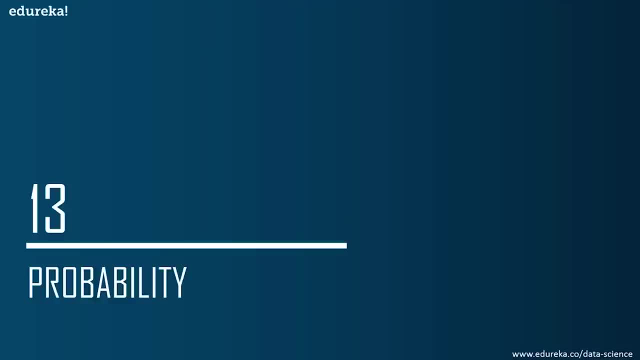 All right. So probability is a mathematical method used for statistical analysis. Therefore, we can say that a probability and statistics are interconnected branches of mathematics that deal with analyzing the relative frequency of events. So they're very interconnected fields and probability makes use of statistics. 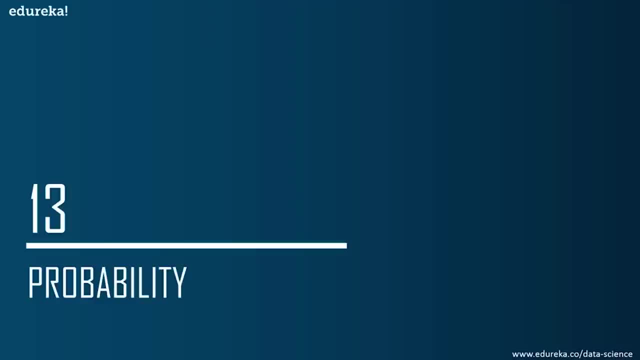 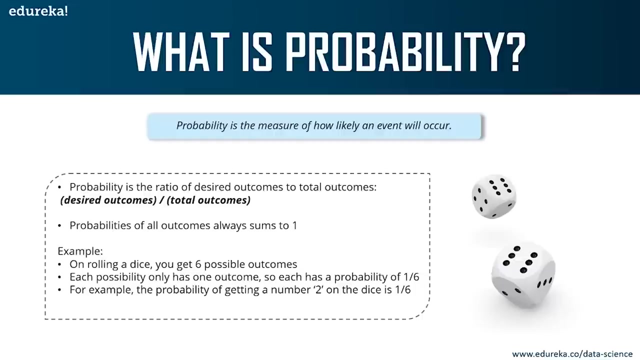 and statistics makes use of probability. All right, they're very interconnected fields. So that is the relationship between statistics and probability. Now let's understand what exactly is probability. So probability is the measure of how likely an event will occur. To be more precise, 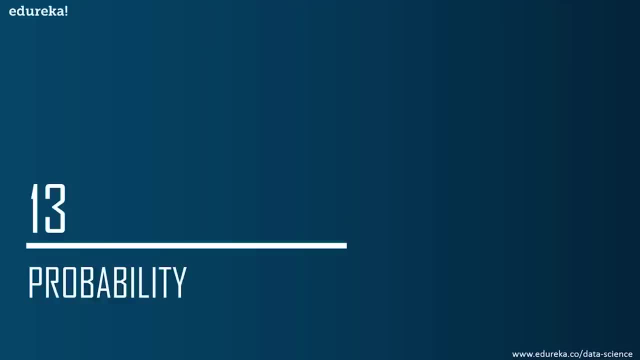 Therefore we can say that a probability and statistics are interconnected branches of mathematics that deal with analyzing the relative frequency of events. So they're very interconnected fields. and probability makes use of statistics and statistics makes use of probability. All right, They're very interconnected fields. 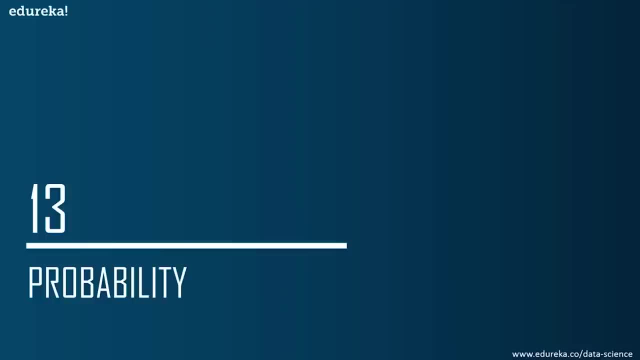 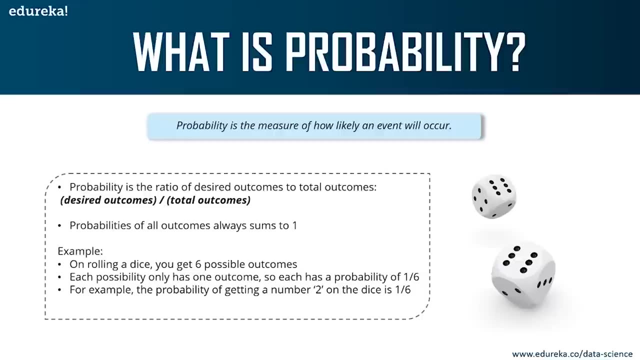 So that is the relationship between statistics and probability. Now let's understand what exactly is probability. So probability is the measure of how likely an event will occur. To be more precise, It is the ratio of desired outcome to the total outcomes. Now, the probability of all outcomes always sum up to one. 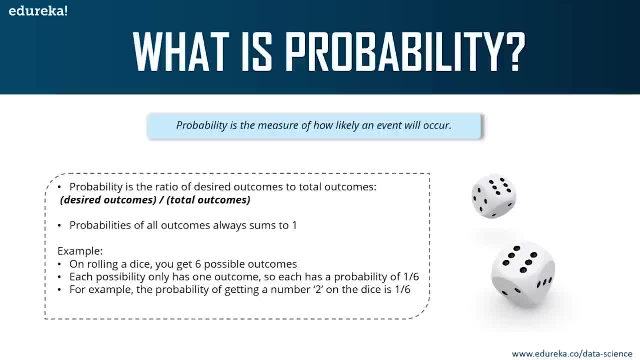 Now the probability will always sum up to one. probability cannot go beyond one. Okay, So either your probability can be zero, or it can be one, or it can be in the form of decimals, like 0.52 or 0.55, or it can be in the form of 0.5, 0.7, 0.9,. 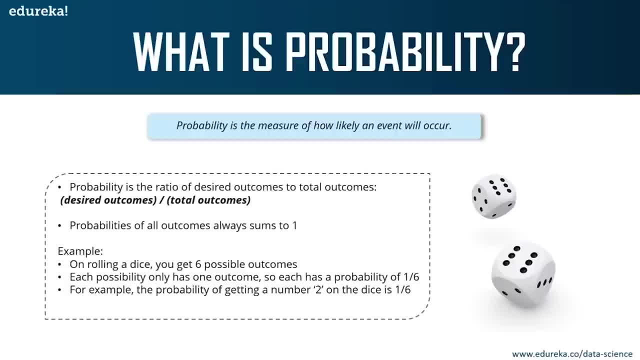 but its value will always stay between the range 0 and 1.. Okay, Now the famous example of probability is rolling a dice example. So when you roll a dice, you get six possible outcomes. right, You get 1, 2, 3, 4 and 5, 6 phases of a dice. 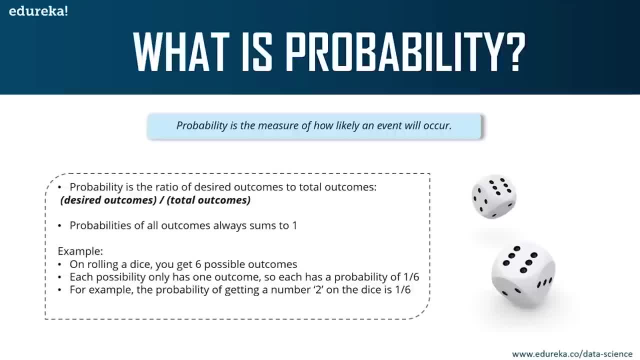 Now, each possibility Only has one outcome. So what is the probability that, on rolling a dice, You'll get 3? the probability is 1 by 6, right, Because there's only one phase which has the number 3 on it out of 6 phases. 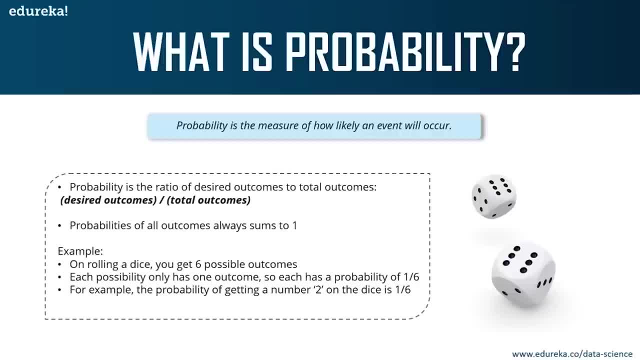 There's only one phase which has the number 3.. So the probability of getting 3 when you roll a dice is 1 by 6.. Similarly, if you want to find the probability of getting a number 5, again the probability is going to be 1 by 6.. 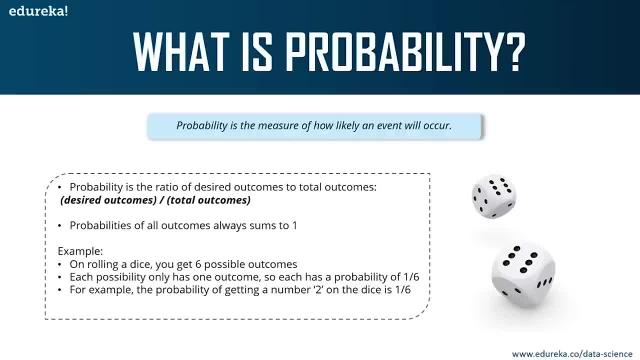 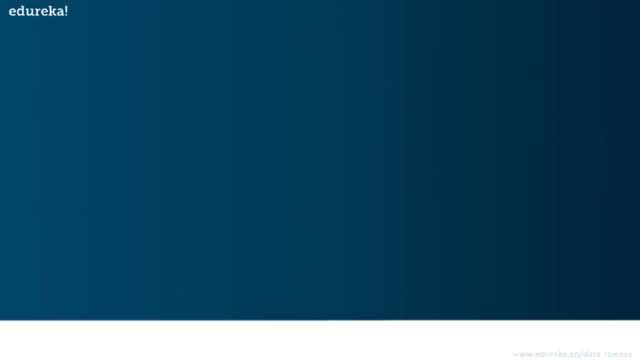 All right, So all of this will sum up to 1. All right. So, guys, this is exactly what probability is. It's a very simple concept. We all learnt it in 8th standard onwards. right Now, let's understand the different terminologies that are related to probability. 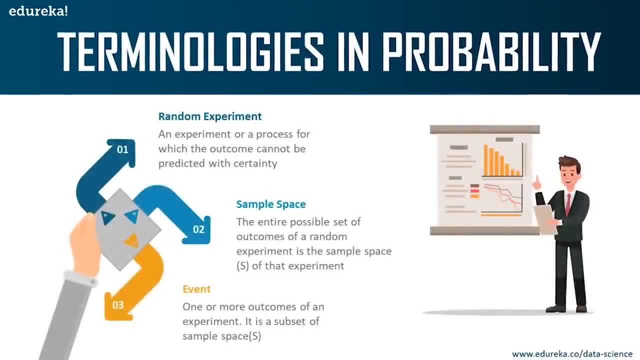 Now, there are three terminologies that you often come across when we talk about probability. We have something known as the random experiment. Okay, It's basically an experiment or a process for which the outcomes cannot be predicted with certainty. All right, That's why you use probability. 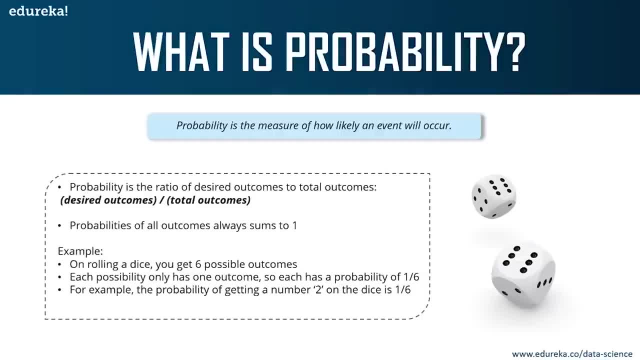 it is the ratio of desired outcome to the total outcomes. Now, the probability of all outcomes always sum up to one. Now, the probability will always sum up to one. Probability cannot go beyond one. Okay, So either your probability can be zero, or it can be one, or it can be in. 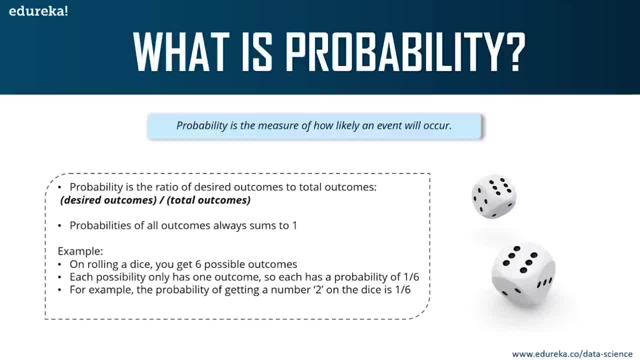 the form of decimals like 0.52 or 0.55, or it can be in the form of 0.5, 0.7, 0.9,, but its value will always stay between the range 0 and 1.. 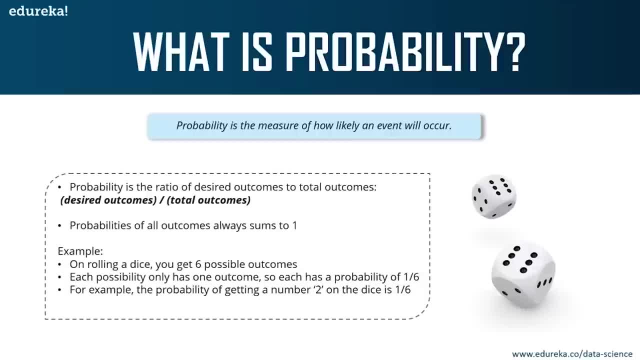 Okay, Now the famous example of probability is rolling a dice example. So when you roll a dice, you get six possible outcomes. right, You get one, two, three, four and five, six phases of a dice. Now, each possibility only has one outcome. 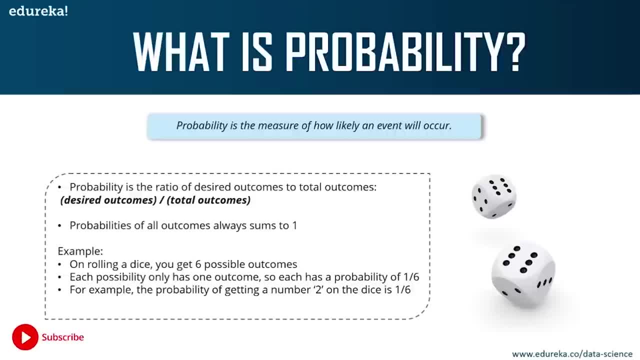 So what is the probability that, on rolling a dice, you'll get three? The probability is one by six, right, Because there's only one phase which has the number three on it. Out of six phases, there's only one phase which has the number three. 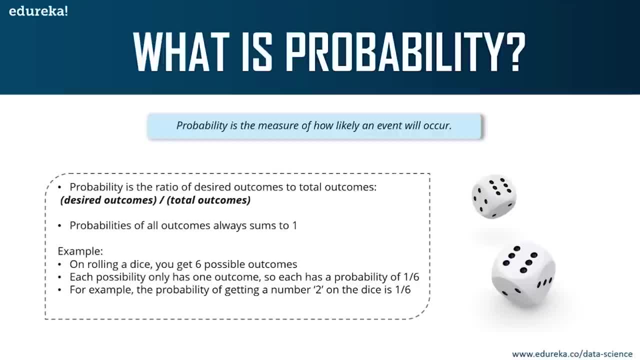 So the probability of getting three when you roll a dice is one by six. Similarly, if you want to find the probability of getting a number five again, the probability is going to be one by six. All right, So all of this will sum up to one. 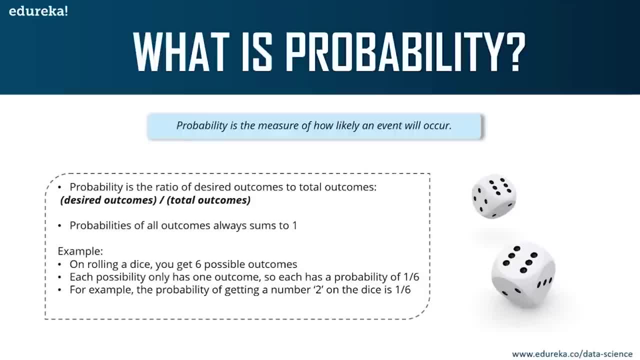 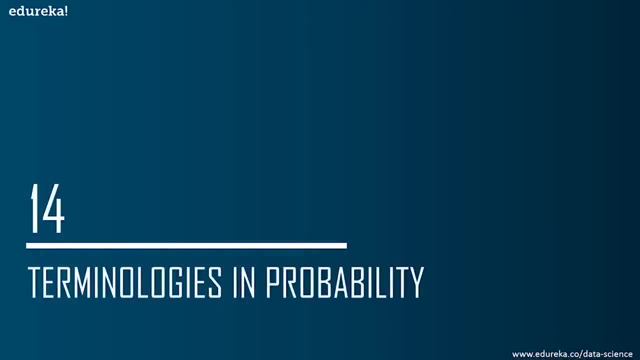 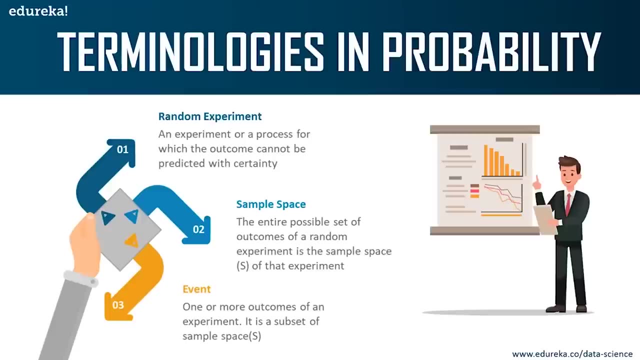 All right. So, guys, this is exactly what probability is. It's a very simple concept. We all learnt it in 8th standard onwards. right Now let's understand the different terminologies that are related to probability. Now there are three terminologies that you often come across when we talk about probability. 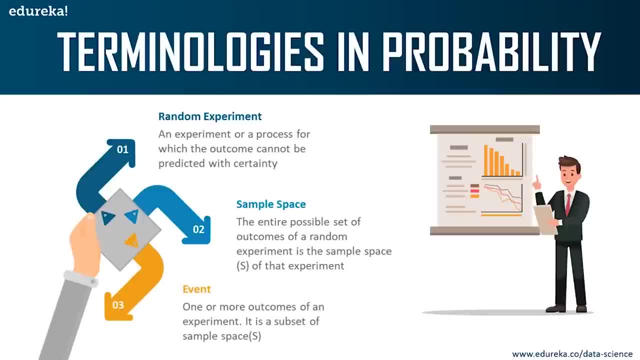 We have something known as the random experiment. It's basically an experiment or a process for which the outcomes cannot be predicted with certainty. All right, that's why you use probability. You're going to use probability in order to predict the outcome with some sort of 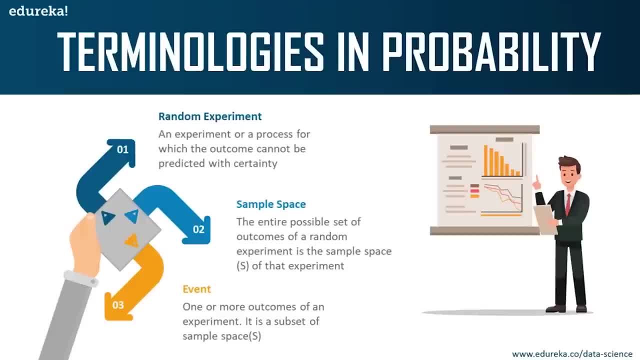 certainty. Sample space is the entire possible set of outcomes of a random experiment. An event is one or more outcomes of an experiment. So if you consider the example of rolling a dice now, let's say that you want to find out the probability. 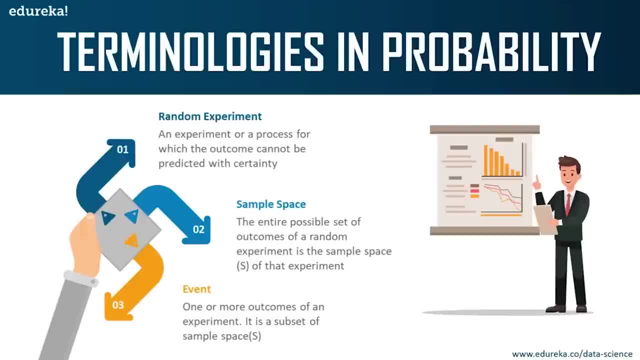 You're going to use probability in order to predict the outcome with some sort of certainty. Sample space is the entire possible set of outcomes of a random experiment. An event is one or more outcomes of an experiment. So if you consider the example of rolling a dice, 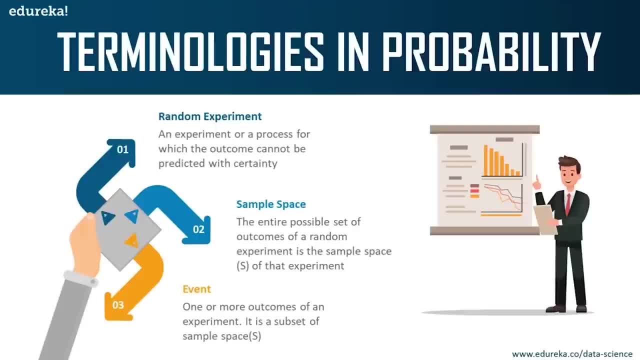 Now let's say that you want to find out the probability of getting a 2 when you roll a dice. Okay, So finding this probability is the random experiment. The sample space Is basically your entire possibility. Okay, So 1, 2,, 3,, 4, 5, 6 phases are there and out of that you need to find the probability of getting a 2.. 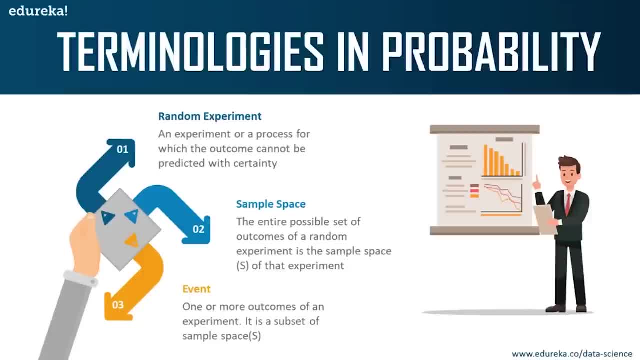 Right, So all the possible outcomes will basically represent your sample space. Okay, So 1 to 6 are all your possible outcomes. This represents your sample space. Now, event is one or more outcome of an experiment. So in this case, my event is to get a 2 when I roll a dice. 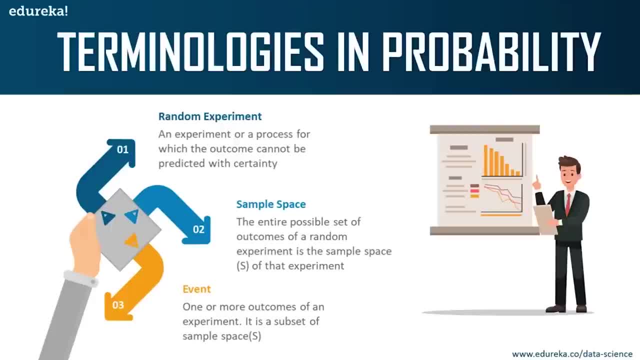 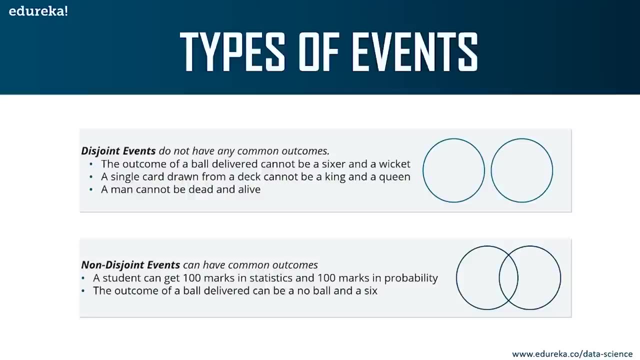 Right. So my event is the probability of getting a 2. When I roll a dice. So, guys, this is basically what random experiment, sample, space and event really means. All right, Now let's discuss the different types of events. There are two types of events that you should know about. 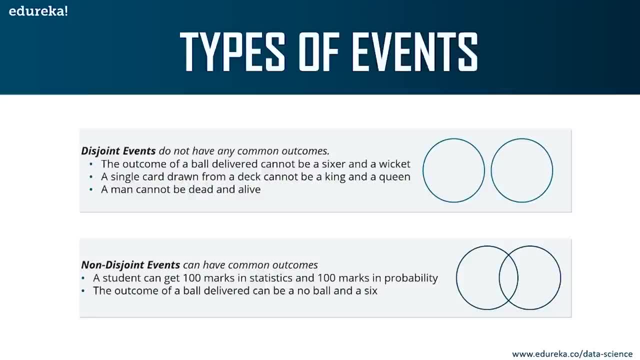 There is disjoint and non disjoint events. Disjoint events are events that do not have any common outcome. For example, if you draw a single card from a deck of cards, it cannot be a king and a queen, Correct, It can either be king. 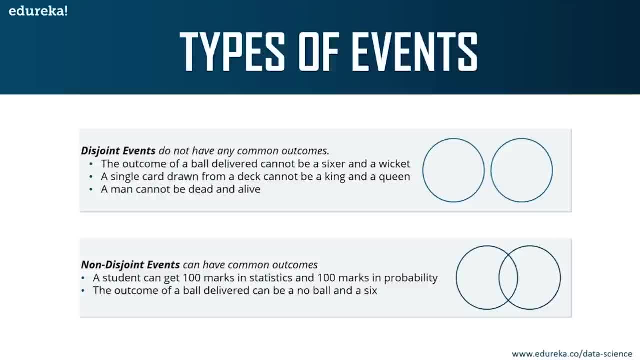 Or it can be queen. Now, non disjoint events are events that have common outcomes. For example, a student can get hundred marks in statistics and hundred marks in probability, All right. And also the outcome of a ball delivered can be a no ball and it can be a 6.. 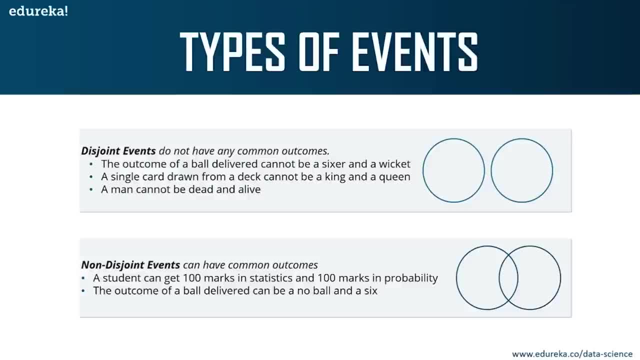 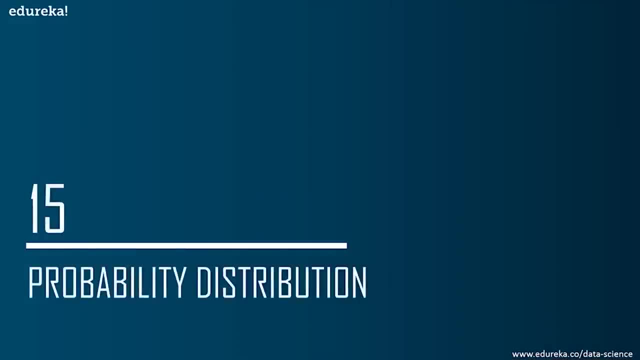 Right. So this is what non disjoint events are. All right, These are very simple to understand Right Now. let's move on and look at the different types of probability distribution. All right, I'll be discussing the three main probability distribution functions. 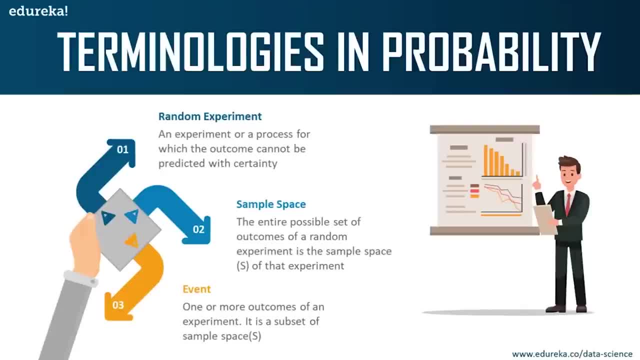 Of getting a two when you roll a dice. Okay, so finding this probability is the random experiment. The sample space is basically your entire possibility. Okay, so one, two, three, four, five, six phases are there and out of that you need to find the probability of getting a. 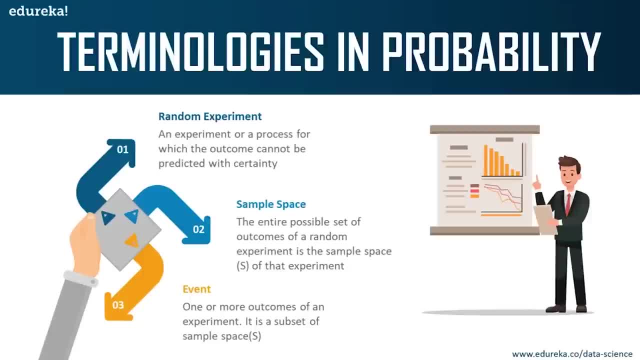 two, right, So all the possible outcomes will basically represent your sample space. Okay, so one to six are all your possible outcomes. This represents your sample space. Now, event is one or more outcome of an experiment. So in this case, my event is to get a two when I roll a dice. 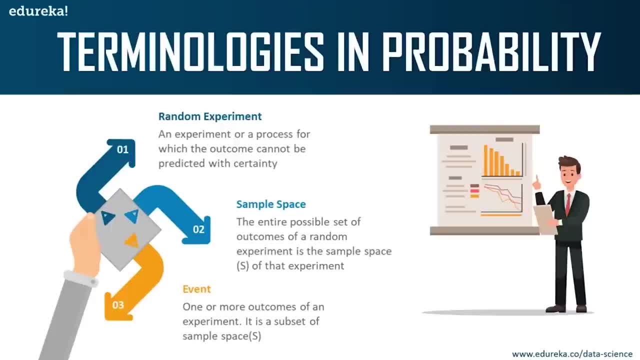 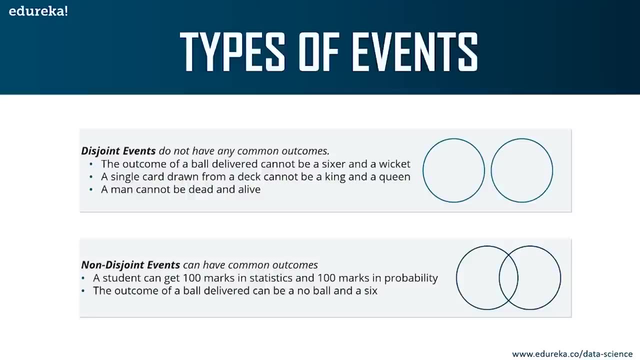 right. So my event is the probability of getting a two when I roll a dice. So, guys, this is basically what random experiment, sample, space and event really means. All right, Now let's discuss the different types of events. There are two types of events that you should know about. 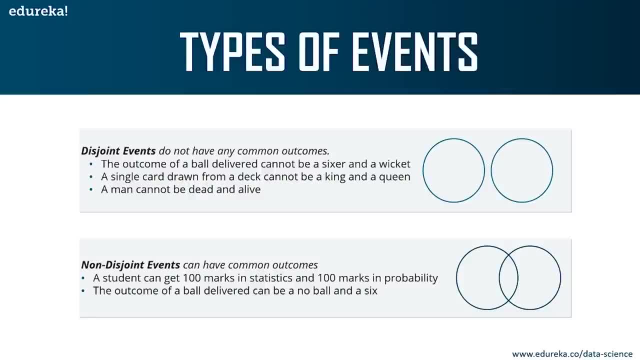 There is disjoint and non disjoint events. Disjoint events are events that do not have any common outcome. For example, if you draw a single card from a deck of cards, it cannot be a king and a queen, correct? It can either be king or it can be queen. 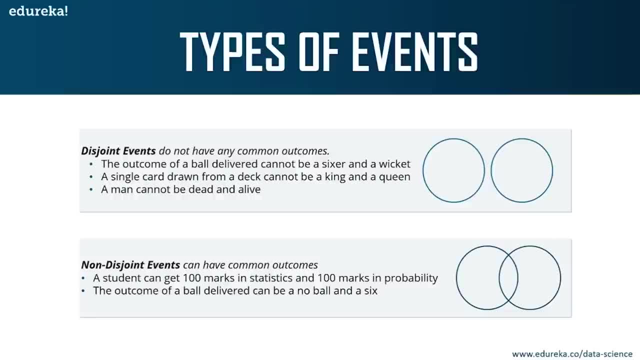 Now, non disjoint events are events that have common outcomes. For example, a student can get hundred marks in statistics and hundred marks in probability, All right. and also the outcome of a ball delivered can be a no ball and it can be a six. 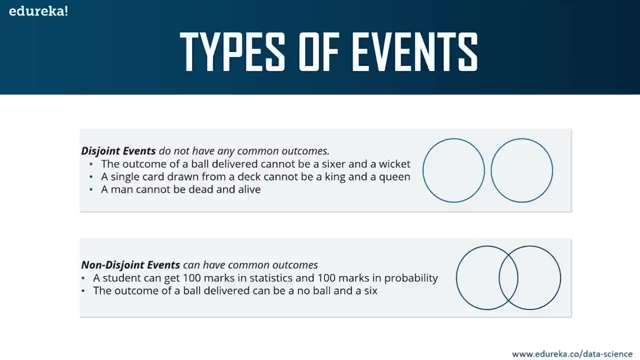 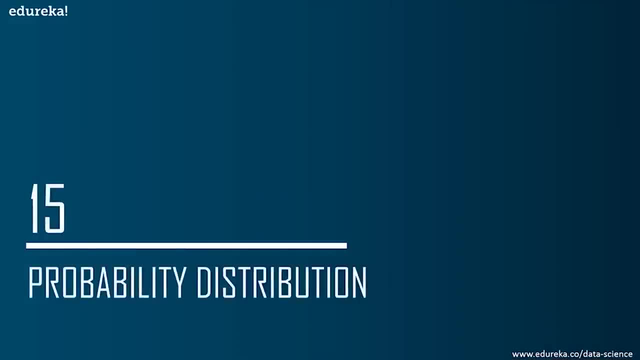 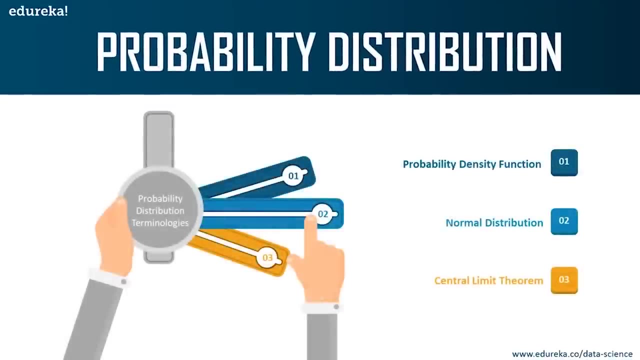 right. So this is what non disjoint events are, and these are very simple to understand Right now. let's move on and look at the different types of probability distribution. All right, I'll be discussing the three main probability distribution functions. I'll be talking about probability density function. 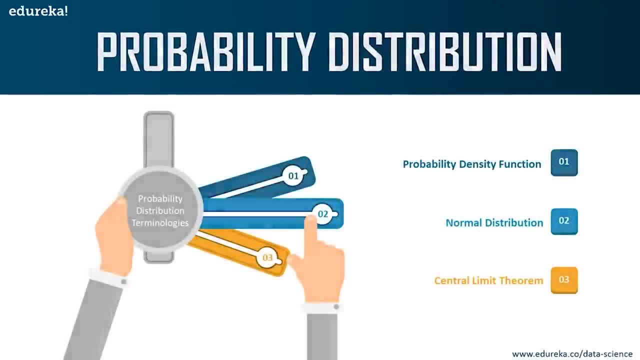 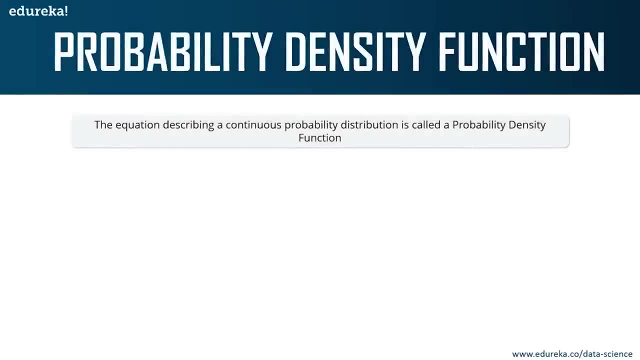 normal distribution and central limit theorem. Okay, probability density function, also known as PDF, is concerned with the relative likelihood for a continuous random variable to take on a given value. All right, So the PDF gives the probability of a variable that lies between the range A and B. 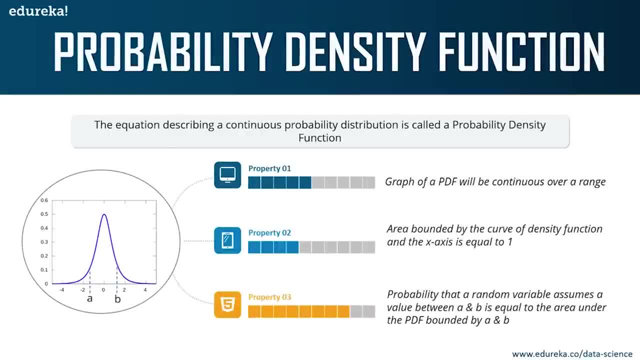 So, basically, what you're trying to do is you're going to try and find the probability of a continuous random variable over a specified range. Okay, Now this graph denotes the PDF of a continuous variable. Now, this graph is also known as the bell curve. 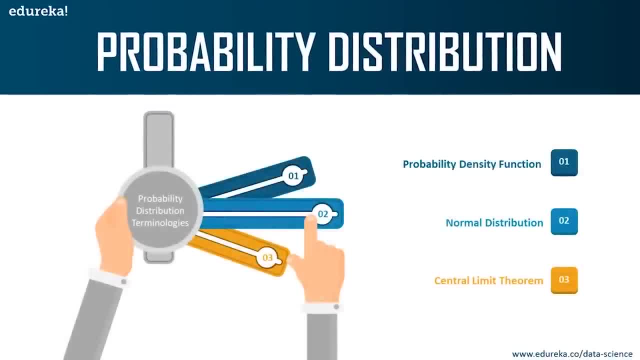 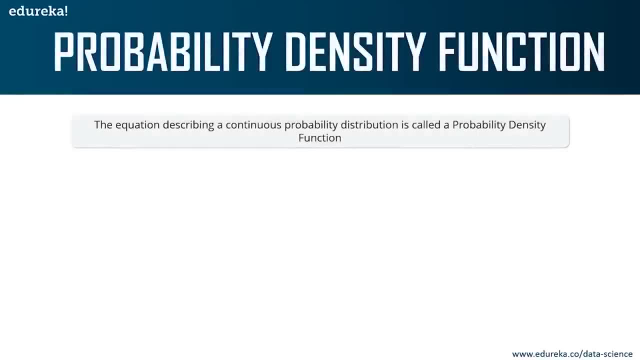 I'll be talking about probability density function, normal distribution and central limit theorem. Okay, Probability density function, also known as PDF, is concerned with the relative likelihood for a continuous random variable to take on a given value. All right, So the PDF gives the probability of a variable that lies between the range A and B. 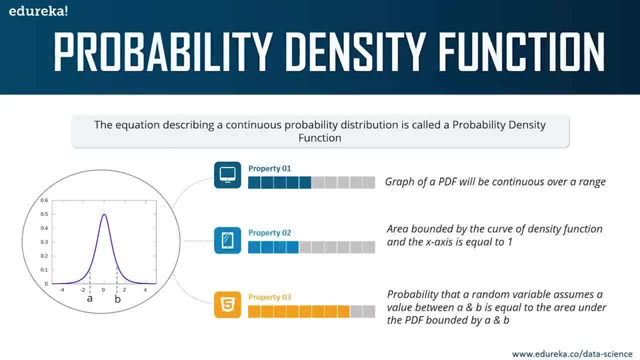 So, basically, what you're trying to do is you're going to Try and find the probability of a continuous random variable over a specified range. Okay, Now this graph denotes the PDF of a continuous variable. Now, this graph is also known as the bell curve. 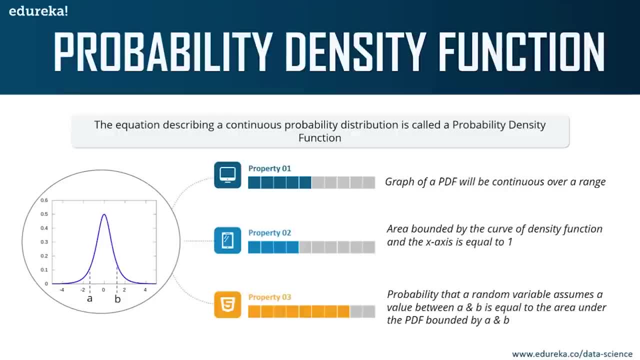 All right. It's famously called the bell curve because of its shape and that three important properties that you need to know about: a probability density function. Now, the graph of a PDF will be continuous over a range. This is because you're finding the probability that a continuous 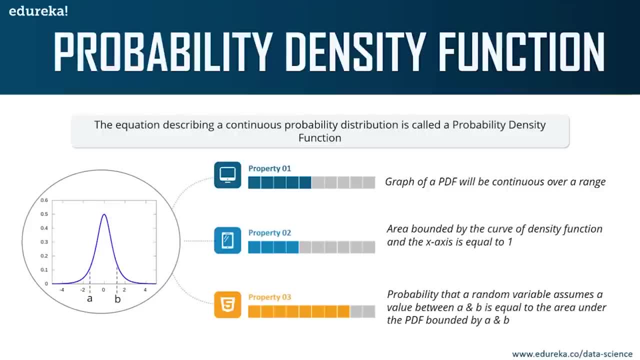 Variable lies between the ranges A and B, Right. The second property is that the area bounded by the curve of a density function and the x-axis is equal to one. Basically, the area below the curve is equal to one. All right, because it denotes probability again. 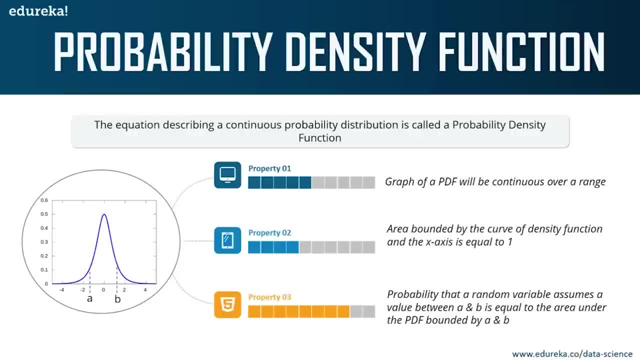 the probability cannot arrange more than one. It has to be between zero and one property. Number three is that the probability that a random variable assumes a value between A and B is equal to the Area under the PDF bounded by A and B. Okay, 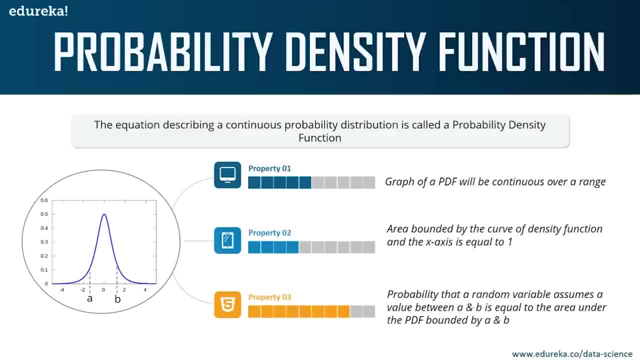 Now, what this means is that the probability value is denoted by the area of the graph, All right. So whatever value that you get here, which basically one, is the probability that a random variable will lie between the range A and B, All right. 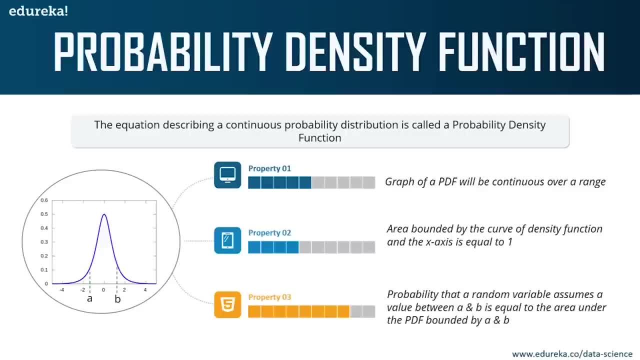 So I hope all of you have understood the probability density function. It's basically the probability of finding the value of a continuous random variable between the range A and B. All right, Now let's look at our next distribution, which is normal distribution. 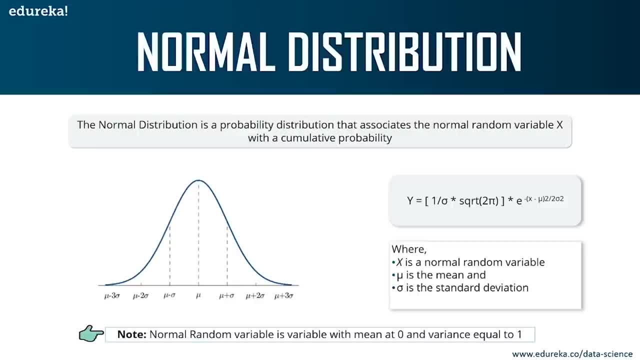 Now, normal distribution, which is also known as the Gaussian distribution, is a probability distribution that denotes the symmetric property of the mean right, Meaning that the idea behind this function is that the data near the mean occurs more frequently than the data away from the mean. 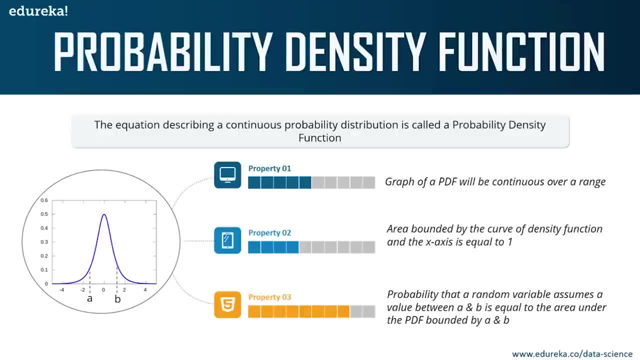 right. It's famously called the bell curve because of its shape, and there are three important properties that you need to know about: a probability density function. Now, the graph of a PDF will be continuous over a range. This is because you're finding the probability that a continuous variable 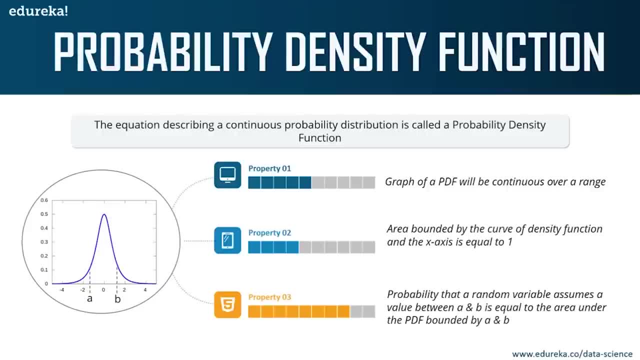 lies between the ranges A and B, right. The second property is that the area bounded by the curve of a density function and the x-axis is equal to one. Basically, the area below the curve is equal to one, All right, because it denotes probability. 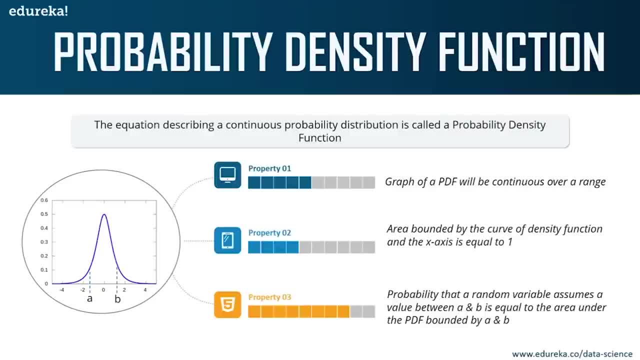 Again, the probability cannot range more than one. It has to be between zero and one Property. number three is that the probability that a random variable assumes a value between A and B is equal to the area under the PDF bounded by A and B. 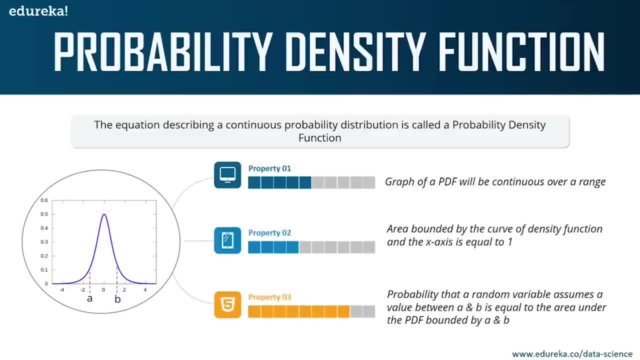 Okay, Now, what this means is that the probability value is denoted by the area of the graph. All right, So whatever value that you get here, which basically one, is the probability that a random variable will lie between the range A and B, 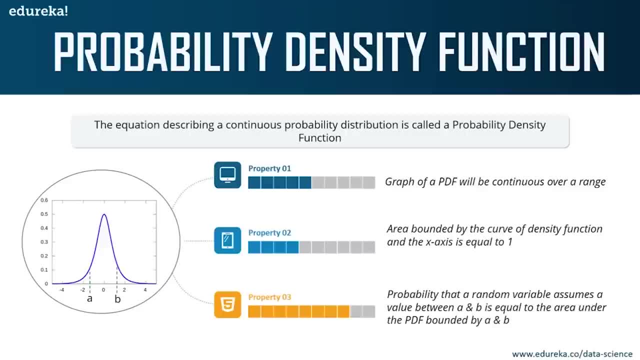 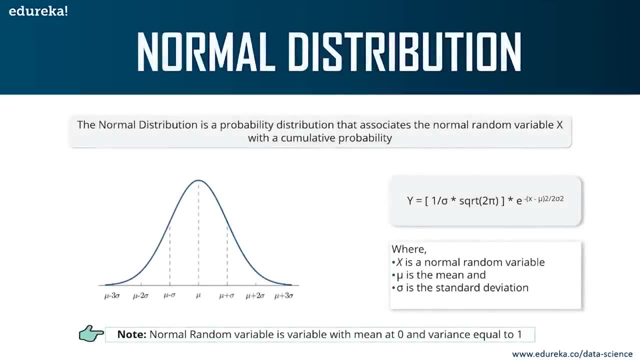 All right, So I hope all of you have understood the probability density function. It's basically the probability of finding the value of a continuous random variable between the range A and B. All right, Now let's look at our next distribution, which is normal distribution. 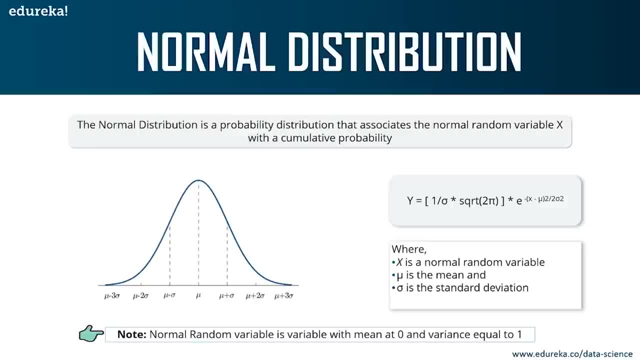 Now, normal distribution, which is also known as the Gaussian distribution, is a probability distribution that denotes the symmetric property of the mean right, Meaning that the idea behind this function is that the data near the mean occurs more frequently than the data away from the mean. 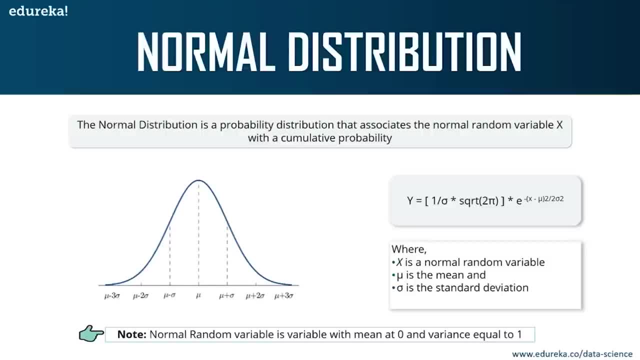 So what it means to say is that the data around the mean represents the entire data set. Okay, So if you just take a sample of data around the mean, it can represent the entire data set. Now, similar to the probability density function, the normal distribution appears as a bell curve. 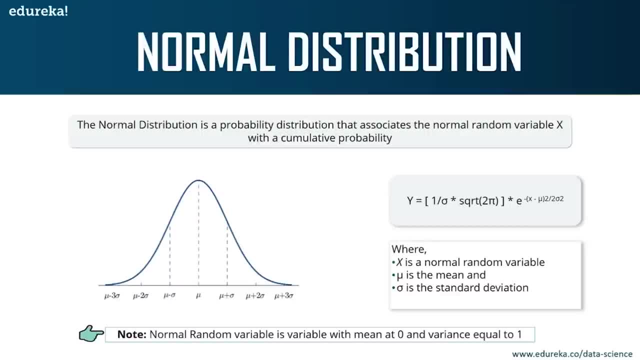 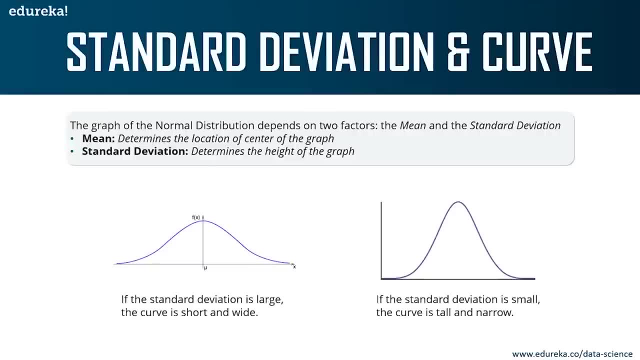 All right. Now, when it comes to normal distribution, there are two important factors. All right, we have the mean of the population and the standard deviation. Okay, So the mean and the graph determines the location of the center of the graph, right? 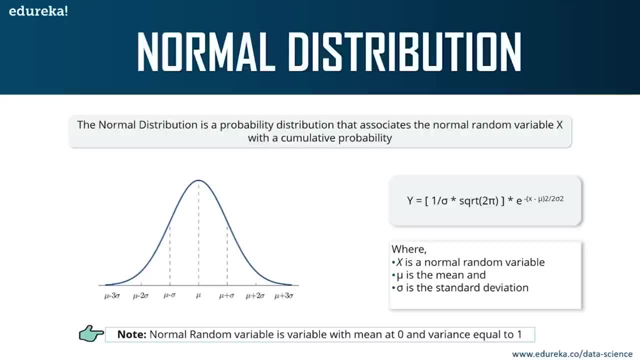 So what it means to say is that the data around the mean represents the entire data set. Okay, So if you just take a sample of data around the mean, it can represent the entire data set. Now, similar to the probability density function, 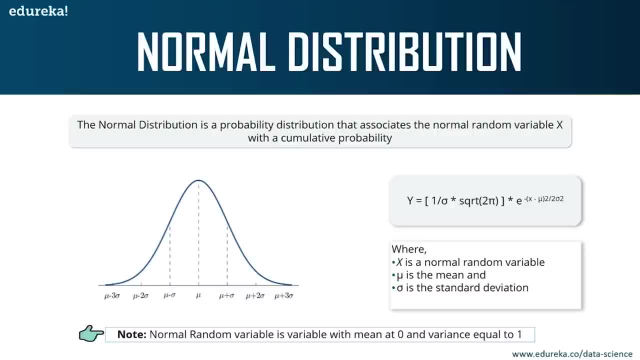 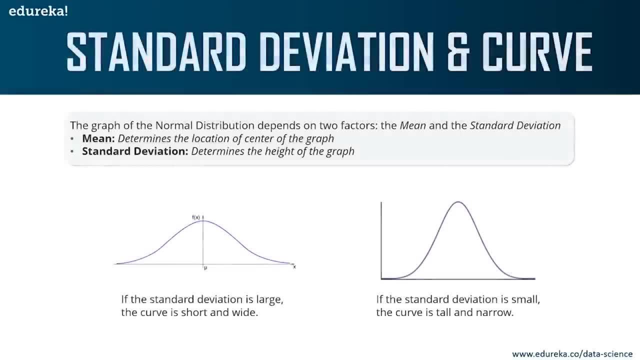 the normal distribution appears as a bell curve. All right. Now, when it comes to normal distribution, there are two important factors. All right, We have the mean of the population and the standard deviation. Okay, So the mean and the graph determines the location of the center of the graph. 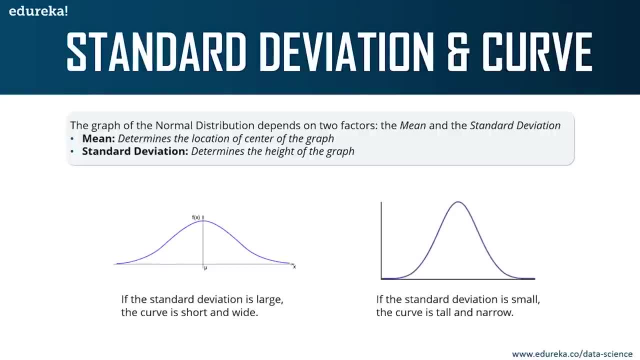 right, And the standard deviation determines the height of the graph. Okay, So if the standard deviation is large, the curve is going to look something like this: All right, it'll be short and wide, And if the standard deviation is small, 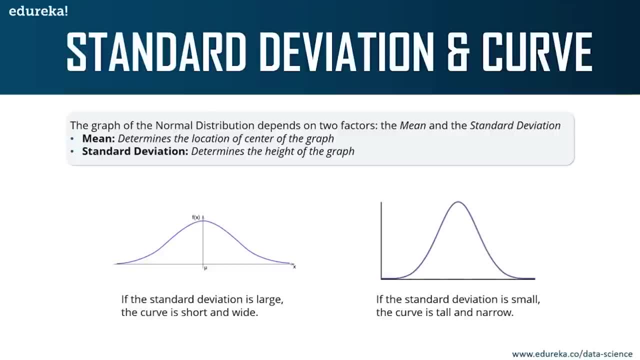 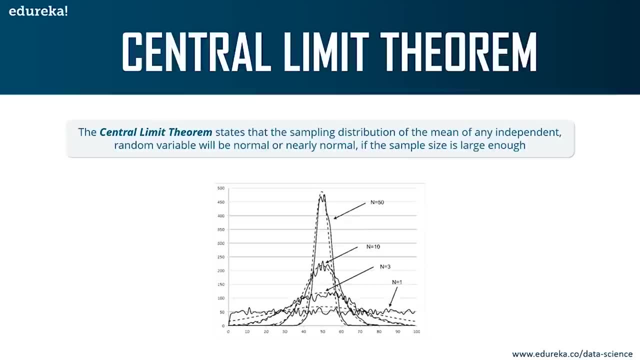 the curve is tall and narrow, All right. So this was it about normal distribution. Now let's look at the central limit theory. Now, the central limit theory states that the sampling distribution of the mean of any independent random variable will be normal or nearly normal if the sample size is large enough. 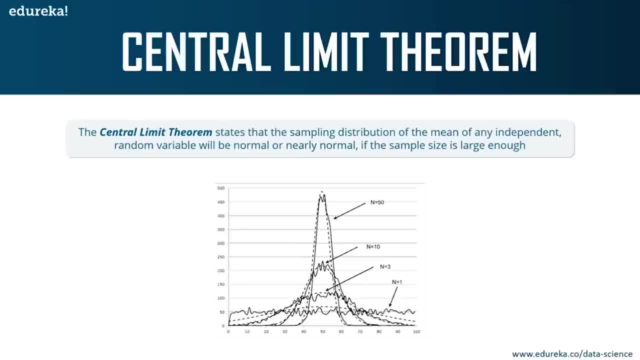 Now that's a little confusing. Okay, let me break it down for you Now in simple terms. if we had a large population and we divided it into many samples, then the mean of all the samples from the population will be almost equal to the mean of the entire population. 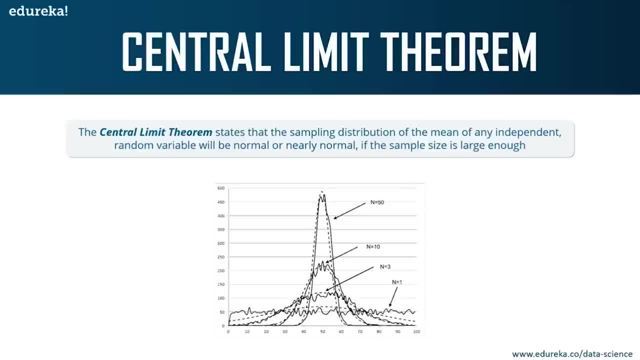 All right, meaning that each of the sample is normally distributed, right? So if you compare the mean of each of the sample, it will almost be equal to the mean of the population, right? So this graph basically shows a more clear understanding of the central limit theorem. 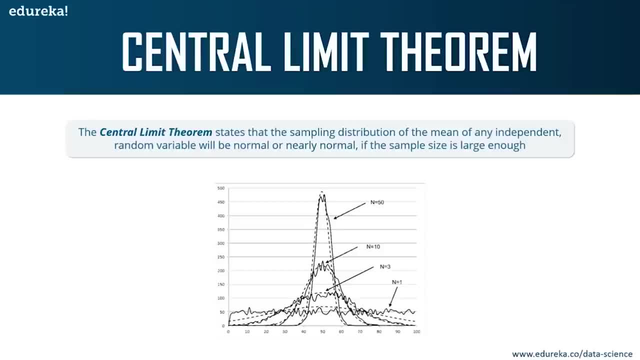 right, You can see each sample here, and the mean of each sample is almost along the same line, right? Okay, So this is exactly what the central limit theorem states. Now, the accuracy or the resemblance to the normal distribution depends on two main factors. 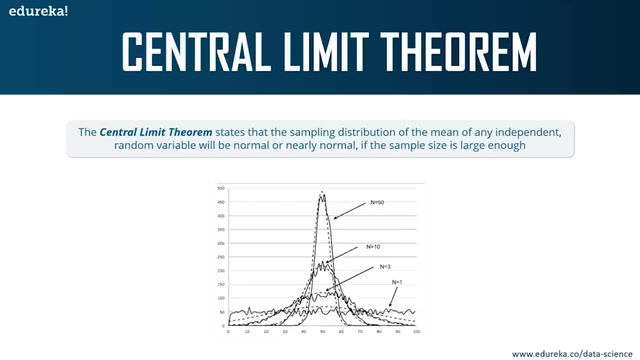 right. So the first is the number of sample points that you consider All right, And the second is the shape of the underlying population. Now, the shape obviously depends on the standard deviation And the mean of a sample, correct? So, guys, 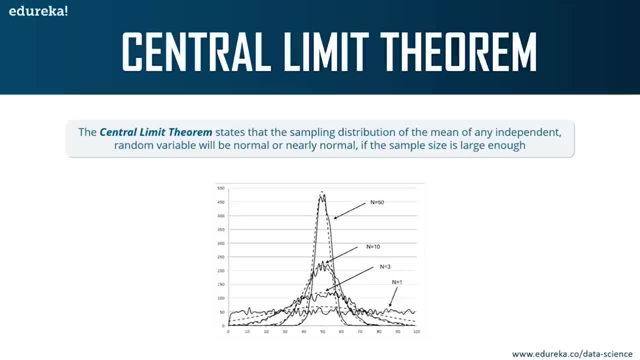 the central limit theorem basically states that each sample will be normally distributed in such a way that the mean of each sample will coincide with the mean of the actual population. All right, in short terms, that's what central limit theorem states. All right. 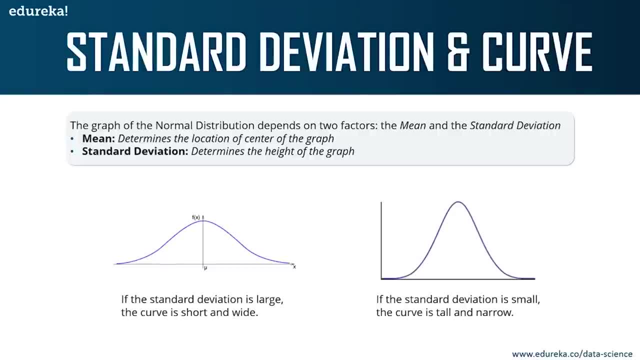 And the standard deviation determines the height of the graph. Okay, So if the standard deviation is large, the curve is going to look something like this: All right, it'll be short and wide, and if the standard deviation is small, the curve is tall and narrow. 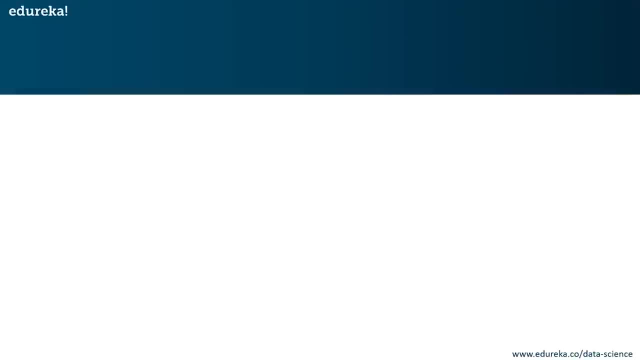 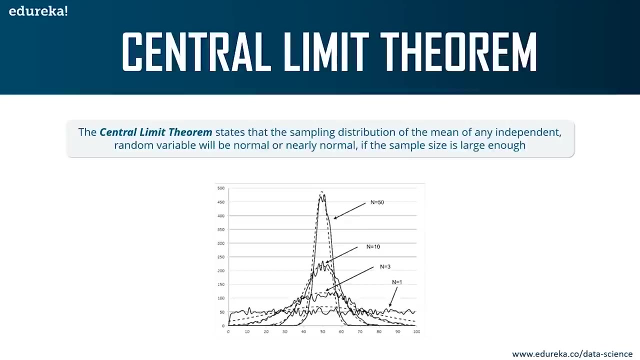 All right, So this was it about normal distribution. Now let's look at the central limit theory. Now, the central limit theory states that the sampling distribution of the mean of any independent random variable will be normal or nearly normal If the sample size is large enough. 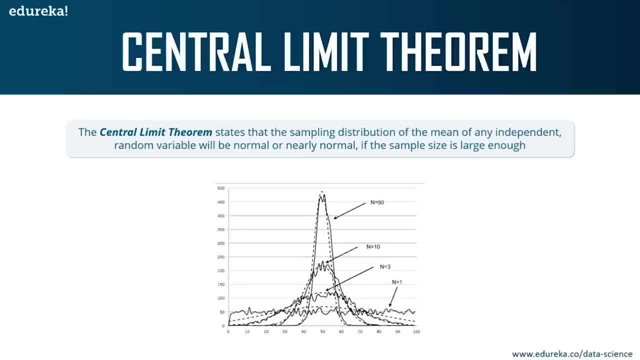 Now that's a little confusing. Okay, let me break it down for you Now in simple terms. if we had a large population and we divided it into many samples, then the mean of all the samples from the population will be almost equal to. 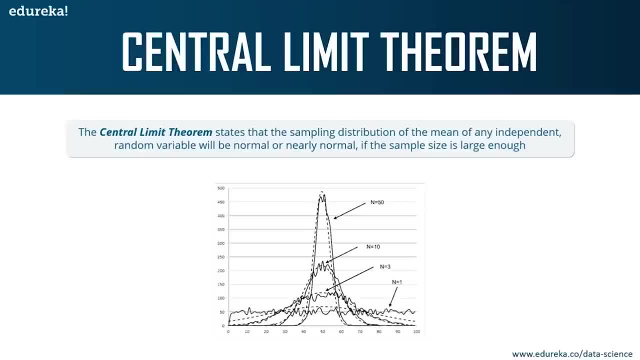 the mean of the entire population, All right, meaning that each of the sample is normally distributed, right? So if you compare the mean of each of the sample, it will almost be equal to the mean of the population, right? So this graph basically shows a more clear understanding of the central limit. 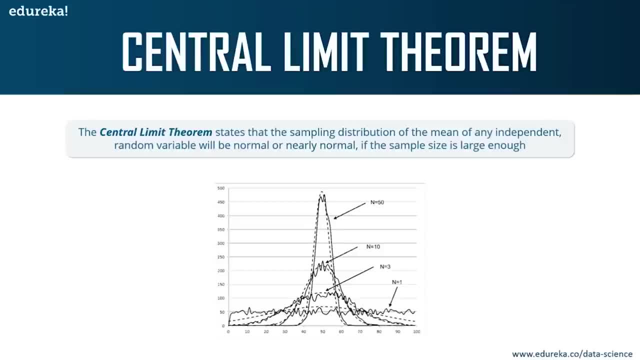 theorem right, You can see each sample here, and the mean of each sample is almost along the same line, right? Okay, So this is exactly what the central limit theorem states. Now, the accuracy or the resemblance to the normal distribution depends on two. 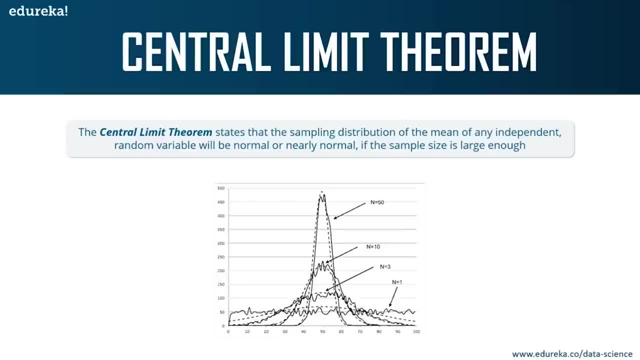 main factors, right? So the first is the number of sample points that you consider All right, and the second is the shape of the underlying population. Now, the shape obviously depends on the standard deviation and the mean of a sample, correct? 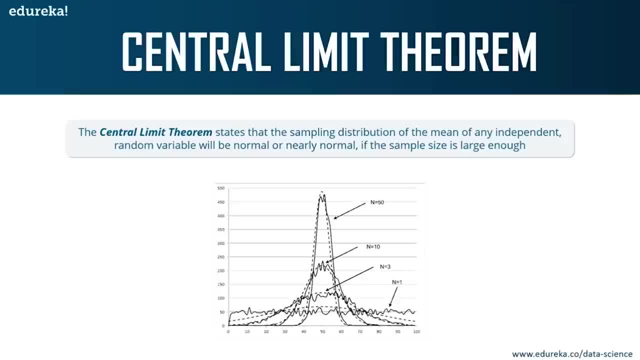 So, guys, the central limit theorem basically states that each sample will be normally distributed in such a way that the mean of each sample will coincide with the mean of the actual population. All right, in short terms, that's what central limit theorem states. 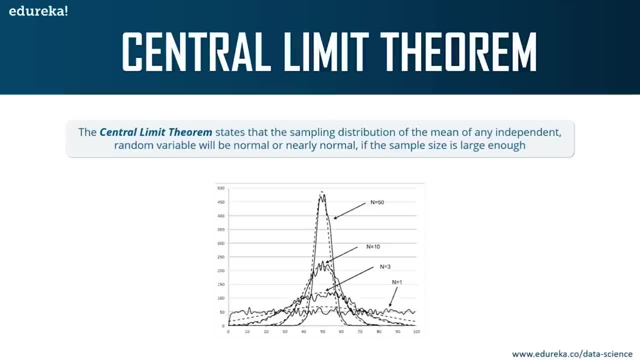 All right, and this holds true only for a large data set, mostly for a small data set, And there are more deviations when compared to a large data set is because of the scaling factor right. The smallest deviation in a small data set will change the value very drastically. 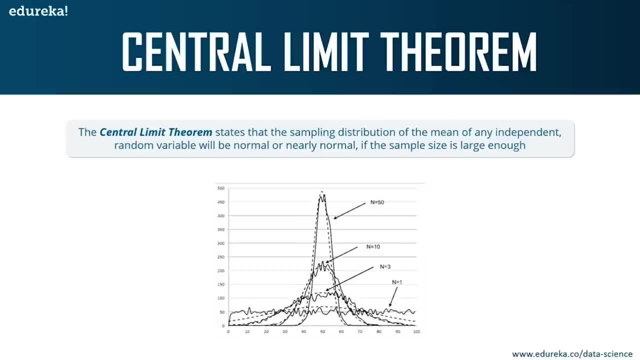 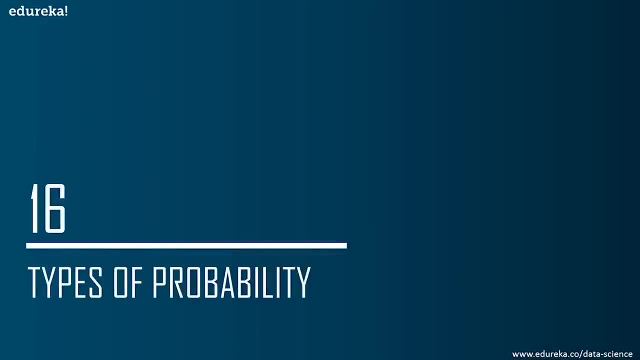 But in a large data set, a small deviation will not matter at all. Now let's move on and look at our next topic, which is the different types of probability. Now, this is a important topic because most of your problems can be solved by understanding. 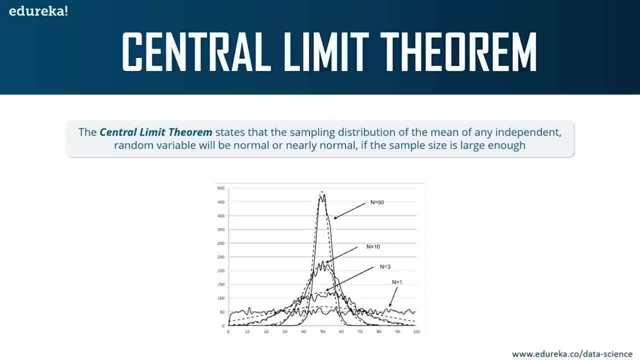 and this holds true only for a large data set, mostly for a small data set, And there are more deviations when compared to a large data set- is because of the scaling factor right. The smallest deviation in a small data set will change The value very drastically. 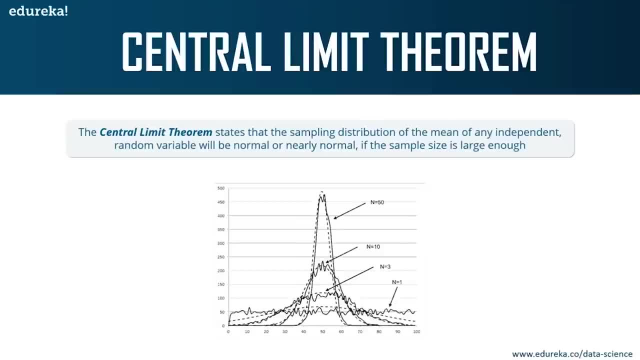 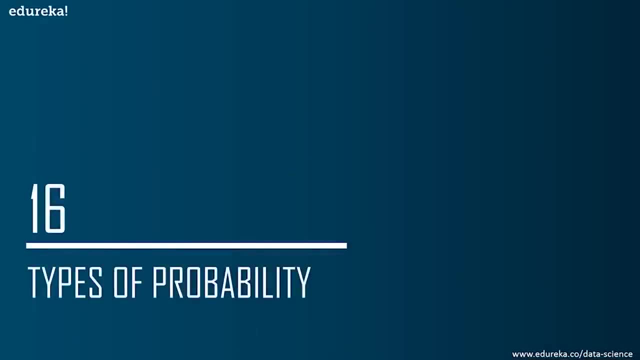 but in a large data set, a small deviation will not matter at all. Now let's move on and look at our next topic, which is the different types of probability. Now, this is a important topic because most of your problems can be solved by understanding which type of probability should I use to solve this problem? 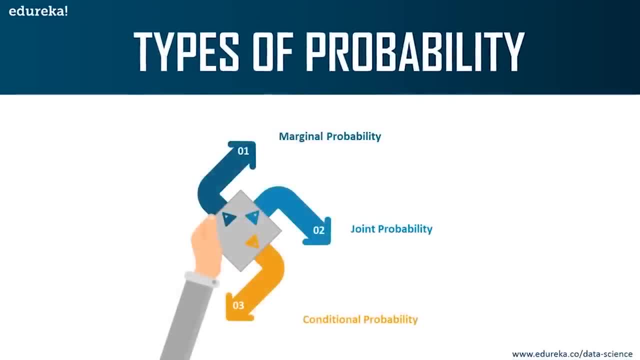 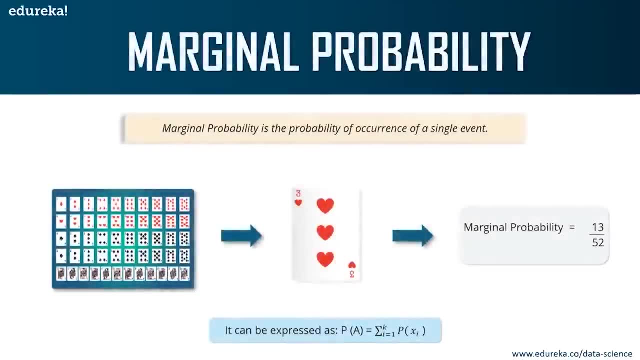 right. So we have three important types of probability. We have marginal, joint and conditional probability. So let's discuss each of these Now. the probability of an event occurring unconditioned on any other event is known as marginal probability or unconditional probability. 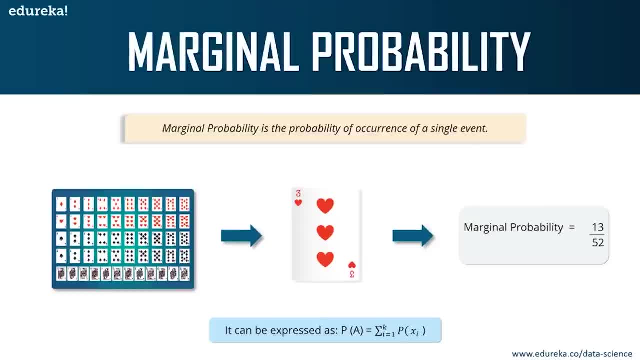 So let's say that you want to find the probability that a card drawn is a heart. All right, So if you want to find the probability that a card drawn is a heart, the probability will be 13 by 52, since there are 52 cards in a deck and there are 13 hearts in a deck of cards. 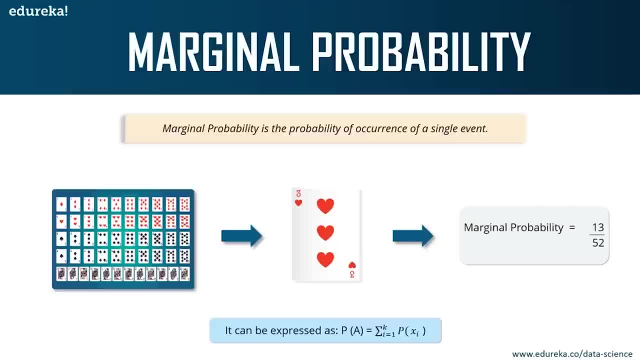 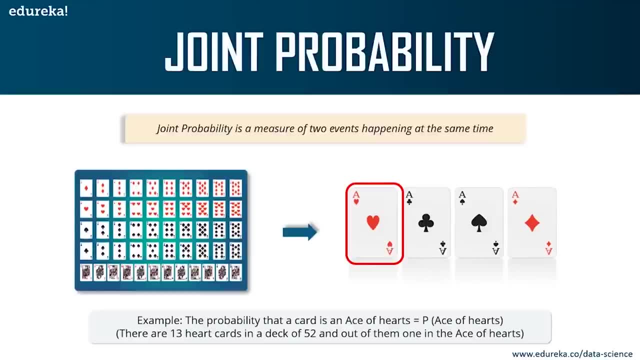 right, And there are 52 cards in a total deck, So your marginal probability will be 13 by 52.. That's about marginal probability. Now let's understand what is joint probability. Now, joint probability is a measure of two events happening at the same time. 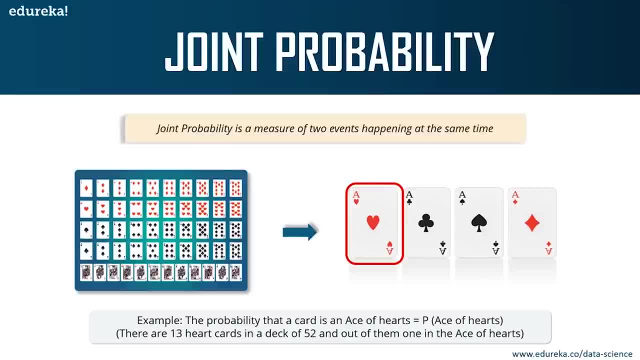 Okay, let's say that the two events are A and B. So the probability of event A and B occurring is the intersection of A and B. So, for example, if you want to find the probability that a card is a 4 and a red, 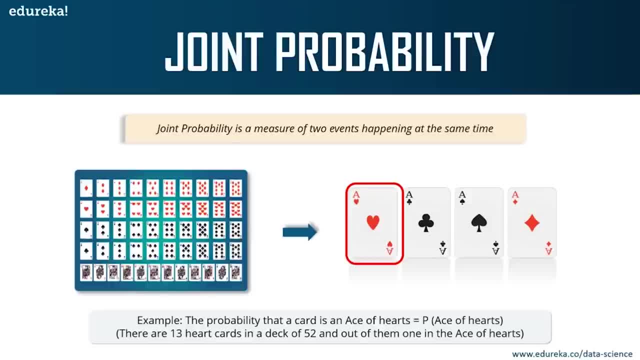 that would be joint probability. All right, because you're finding a card that is 4 and the card has to be red in color. So for the answer, this will be 2 by 52, because we have 1,, 2 in hearts and we have 1,. 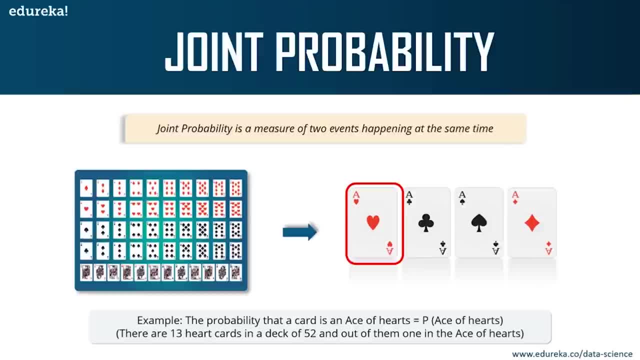 2 in diamonds, correct? So both of these are red in color. Therefore, our probability is 2 by 52. And if you further down it, it is 1 by 26,, right? So this is what joint probability is all about. 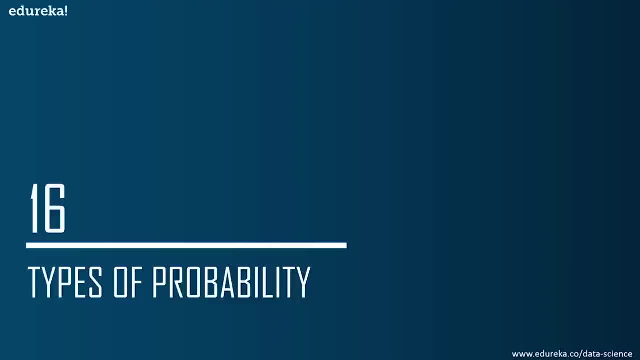 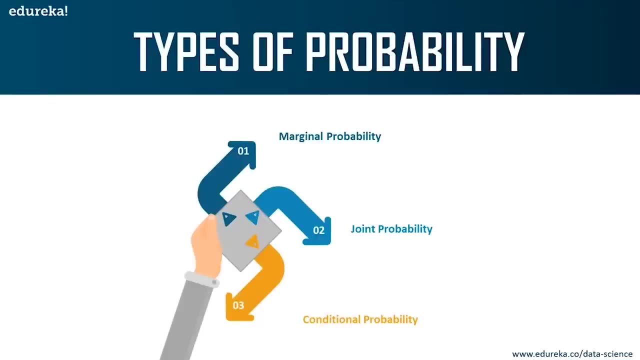 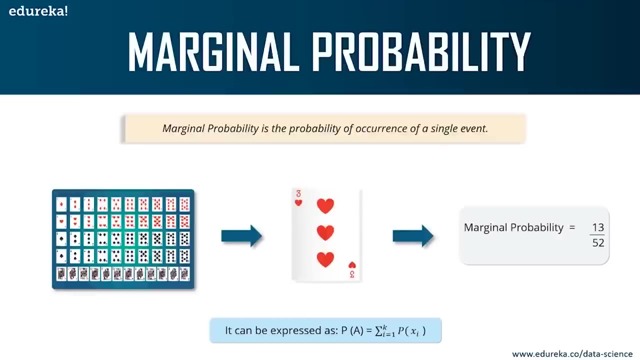 which type of probability should I use to solve this problem? Right, So we have three important types of probability. We have marginal, joint and conditional probability, So let's discuss each of these Now. the probability of an event occurring unconditioned on any other event is known. 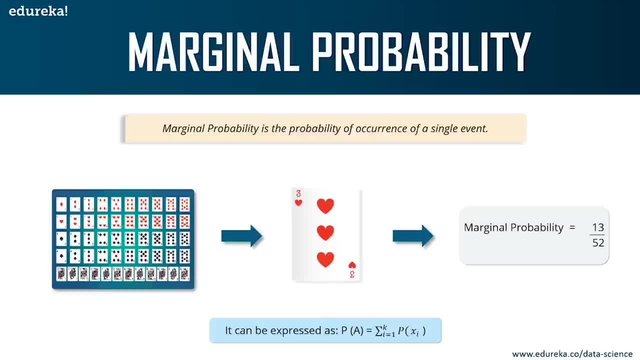 as marginal probability or unconditional probability. So let's say that you want to find the probability that a card drawn is a heart, All right. So if you want to find the probability that a card drawn is a heart, the probability will be 13 by 52.. 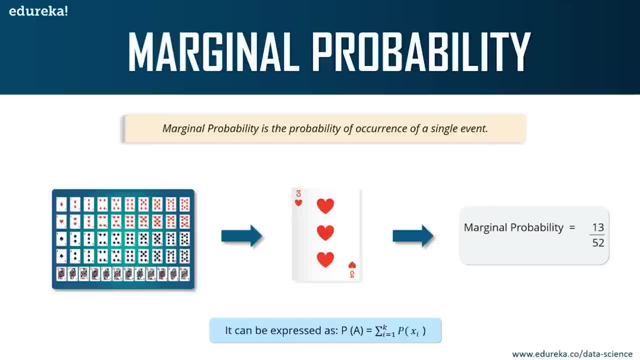 Since there are 52 cards in a deck and there are 13 hearts in a deck of cards right And there are 52 cards in a total deck, So your marginal probability will be 13 by 52.. That's about marginal probability. 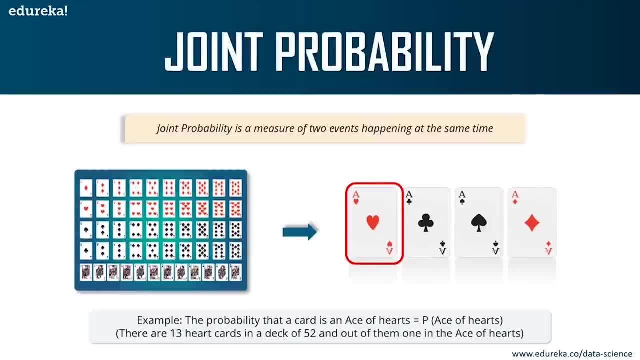 Now let's understand what is joint probability. Now, joint probability is a measure of two events happening at the same time. Okay, let's say that the two events are A and B. So the probability of event A and B occurring is the intersection. 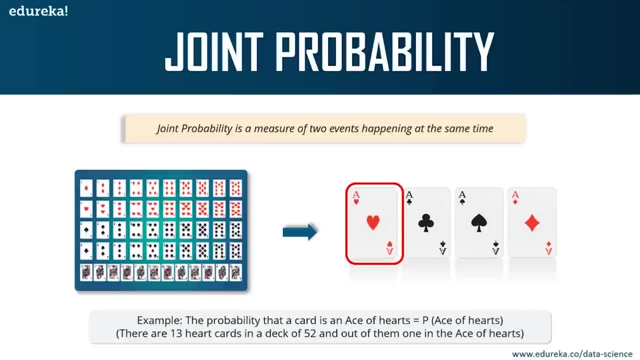 Of A and B. So, for example, if you want to find the probability that a card is a four and red, that would be joint probability, All right, because you're finding a card that is four and the card has to be red in color. 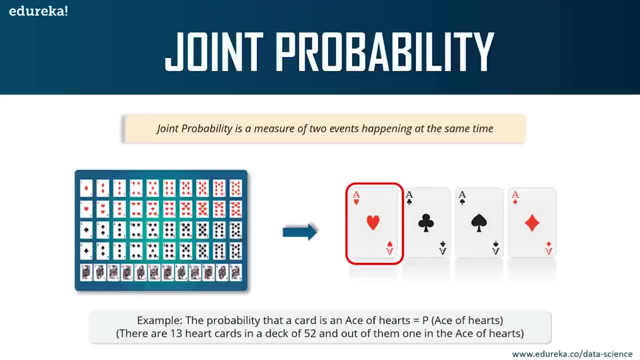 So for the answer, this will be two by 52, because we have one, two in hearts and we have one, two in diamonds, Correct? So both of these are red in color. Therefore, our probability is two by 52. and if you further down it, 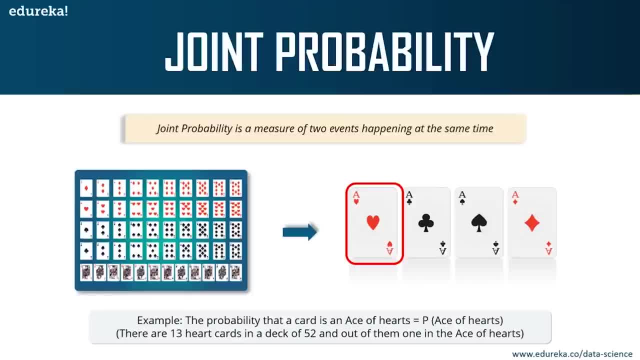 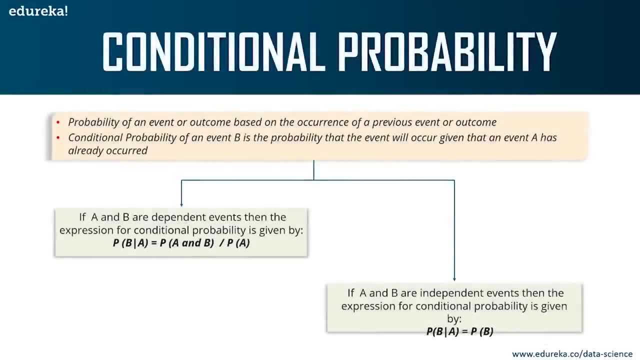 it is one by 26.. Right, So this is what joint probability is all about. moving on, Let's look at what exactly conditional probability is. So if the probability of an event or an outcome is based on the occurrence of a previous event or an outcome, 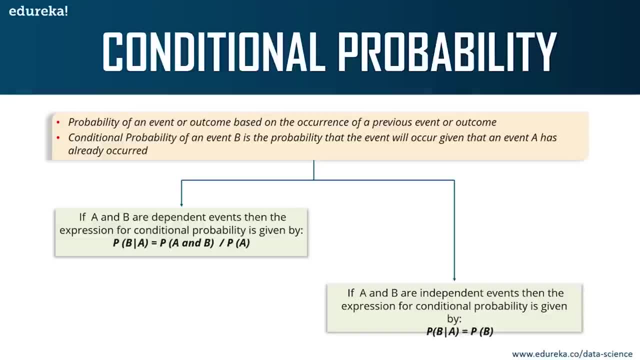 then you called it as a conditional probability. Okay, So the conditional probability of an event B is the probability that the event will occur, given that an event A has already occurred. Right? So if A and B are dependent events, then the expression for conditional probability is given by this. 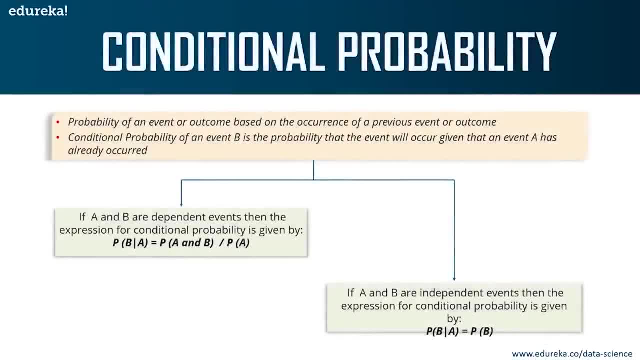 Moving on, Let's look at what exactly conditional probability is. So if the probability of an event or an outcome is based on the occurrence of a previous event or an outcome, then you called it as a conditional probability. Okay, so the conditional probability of an event B is the probability that the event 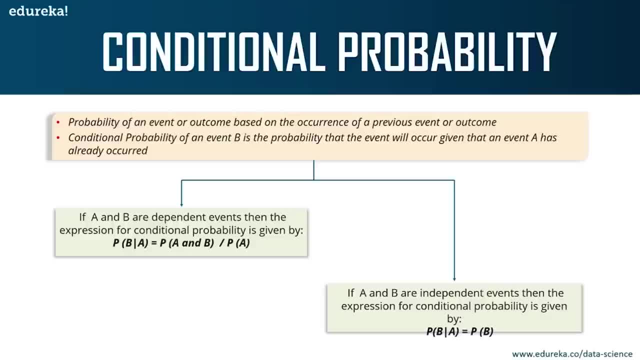 will occur, given that an event A has already occurred, right? So if A and B are dependent events, then the expression for conditional probability is given by this. Now, this first term on the left hand side, which is P, B of A, is basically the probability of event B occurring, given that event. 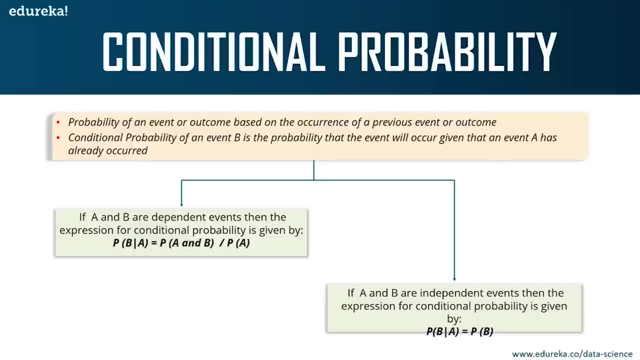 A has already occurred, All right. So, like I said, if A and B are dependent events, then this is the expression, But if A and B are independent events, then the expression for conditional probability is like this: right, So, guys. 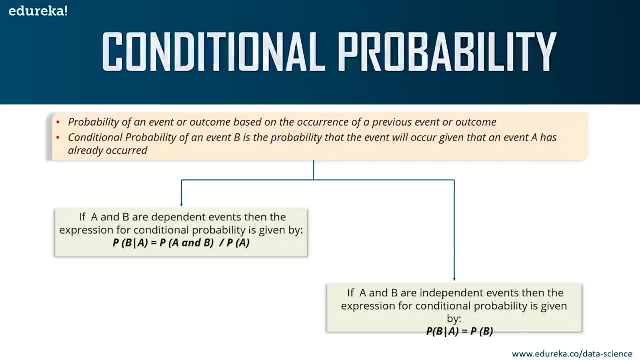 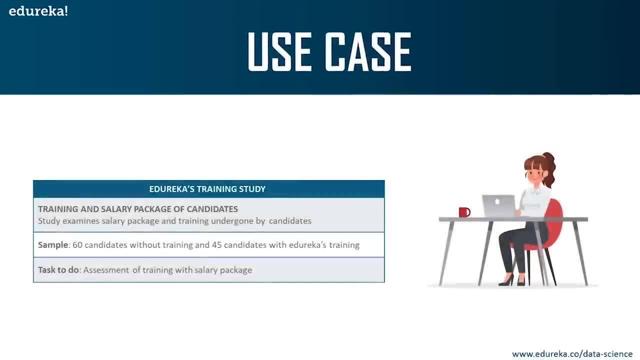 P of A and P of B is obviously the probability of A and probability of B, right Now. let's move on. Now, in order to understand conditional probability, joint probability and marginal probability, let's look at a small use case. 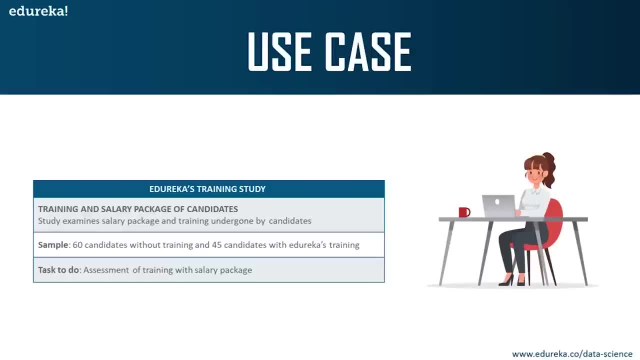 Okay, Now, basically, we're going to take a data set which examines the salary package and training undergone by candidates. Okay, Now, in this there are 60 candidates without training and 45 candidates which have enrolled for Edureka's training right. 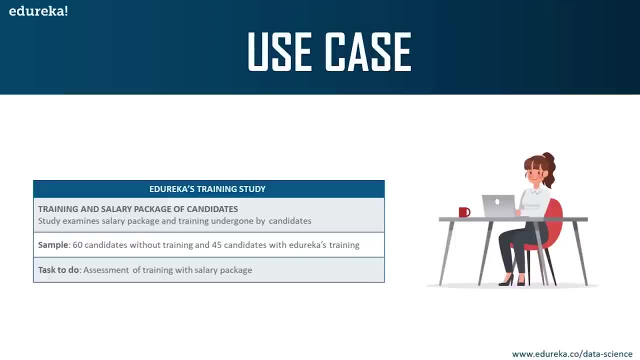 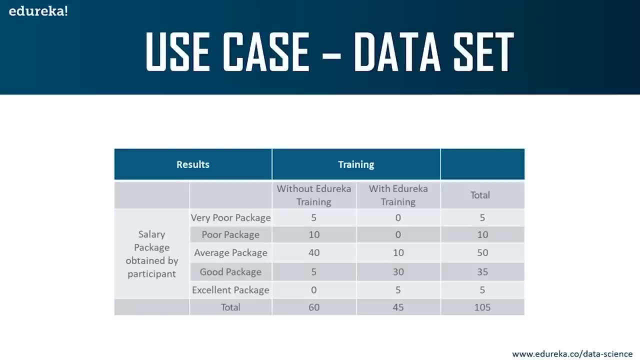 Now the task here is: you have to assess the training with a salary package. Okay, let's look at this in a little more depth. So in total, we have 105 candidates, out of which 60 of them have not enrolled for Edureka's. 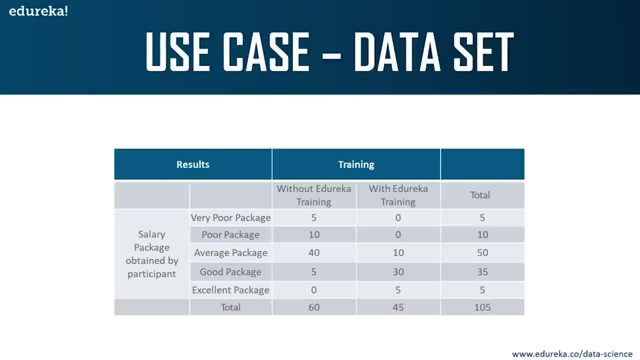 training and 45 of them have enrolled for Edureka's training. All right, This is a small survey that was conducted and this is the rating of the package or the salary that they got right. So if you read through the data, you can understand. there were five candidates without Edureka training who 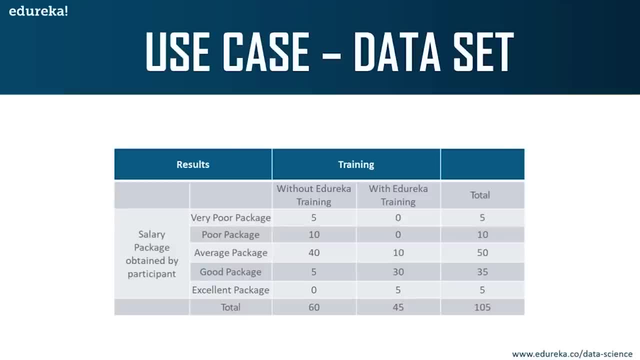 got a very poor salary package Okay. Similarly, there are 30 candidates with Edureka training who got a good package right. So, guys, basically you're comparing the salary package of a person depending on whether or not they've enrolled for Edureka training. 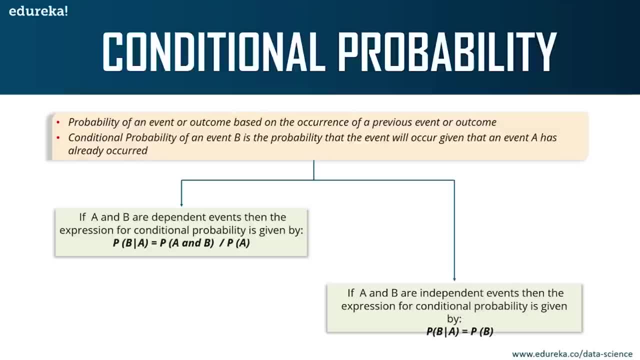 Now, this first term on the left hand side, which is P, B of A is basically the probability of event B occurring, given that event A has already occurred. All right, So, like I said, if A and B are dependent events, then this is the expression. 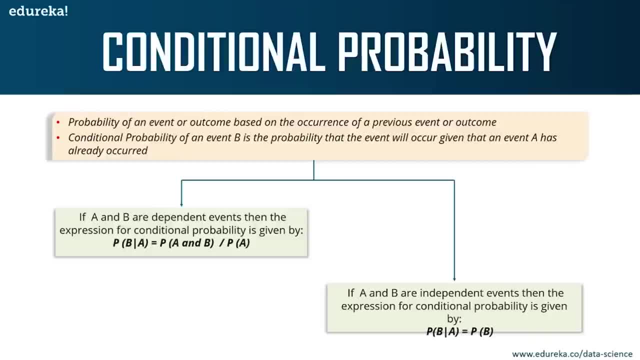 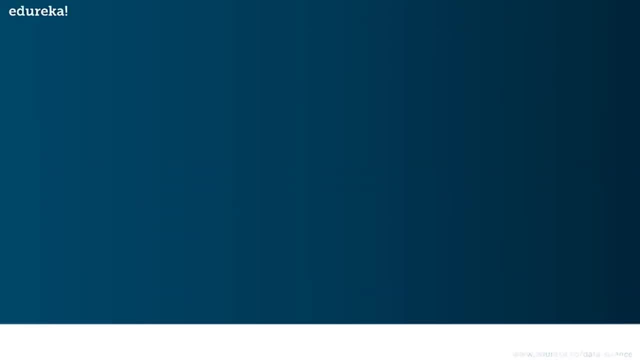 But if A and B are independent events, then the expression for conditional probability is like this: Right, So, guys, P of A and P of B is obviously the probability Of A and probability of B. Right Now, let's move on. 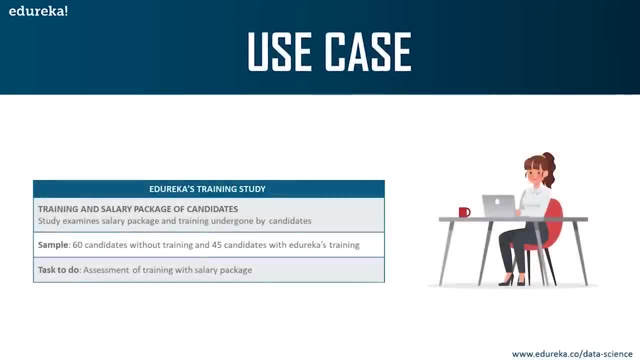 Now, in order to understand conditional probability, joint probability and marginal probability, Let's look at a small use case. Okay, Now, basically, we're going to take a data set which examines the salary package and training undergone by candidates. Okay, Now, in this there are 60 candidates without training and 45 candidates which have enrolled for Edureka's training. 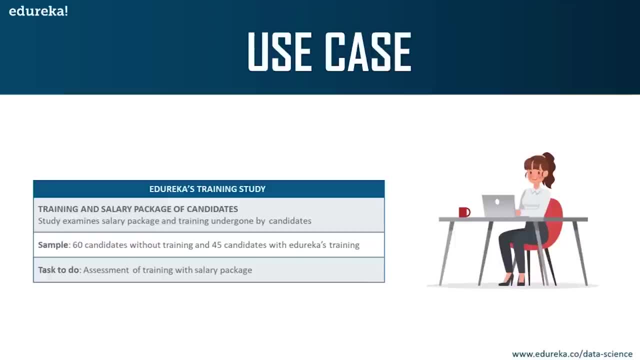 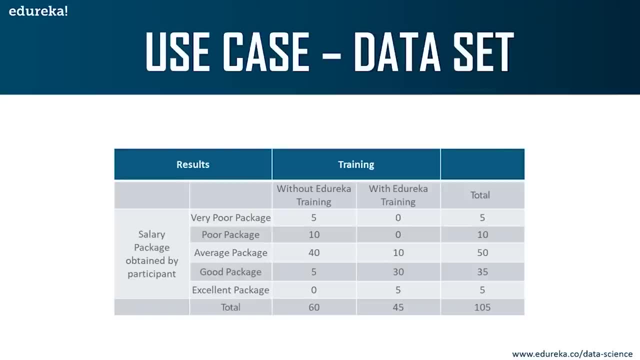 Right Now. the task here is: you have to assess the training with a salary package. Okay, let's look at this in a little more depth. So in total, we have 105 candidates, out of which 60 of them have not enrolled for Edureka's training and 45 of them have enrolled for Edureka's training. 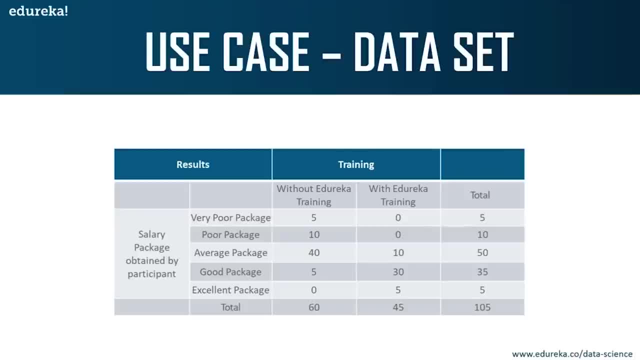 All right, This is a small survey that was conducted and this is the rating of the package or the salary that they got Right. So if you read through the data you can understand. there were five candidates- It's without Edureka training- who got a very poor salary package. 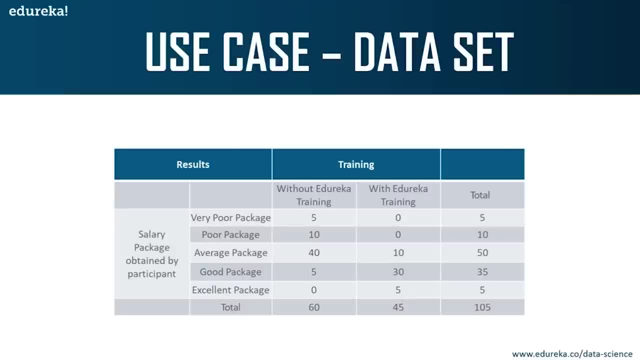 Okay. Similarly, there are 30 candidates with Edureka training who got a good package, Right? So, guys, basically you're comparing the salary package of a person depending on whether or not they've enrolled for Edureka training, Right? This is our data set. 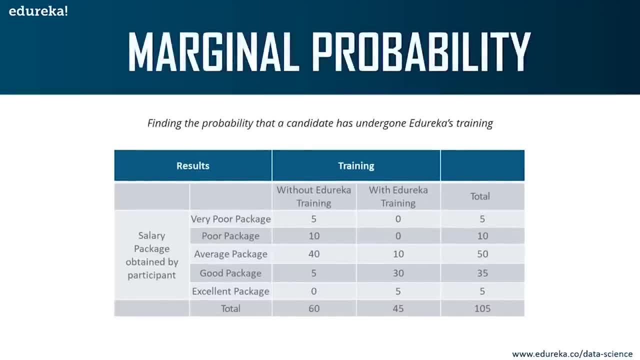 Now let's look at a problem statement. Find the probability that a candidate has undergone Edureka's training Quite simple. Which type of probability is this? This is marginal probability, Right? So the probability that a candidate has undergone Edureka's training is obviously 45 divided by 105.. 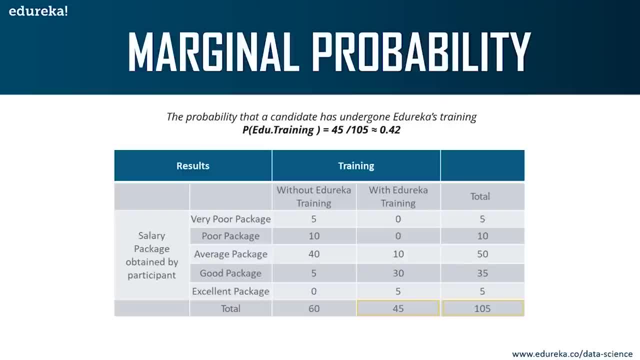 Since 45 is the number of candidates with Edureka training and 105 is the total number of candidates, So you get a value of approximately 0.42.. All right, that's the probability of a candidate that has undergone Edureka's training. 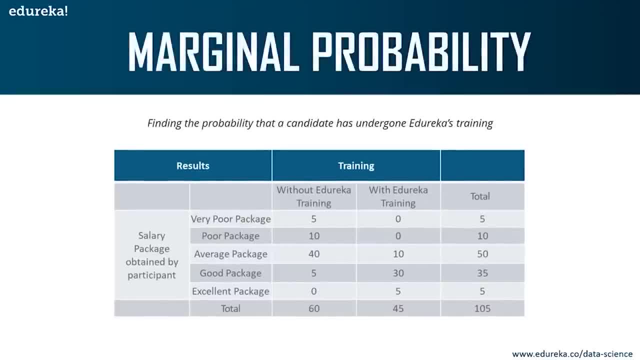 right, This is our data set. Now let's look at our problem statement. Find the probability that a candidate has undergone Edureka's training Quite simple. Which type of probability is this? This is marginal probability, right? So the probability that a candidate has undergone Edureka's training is obviously. 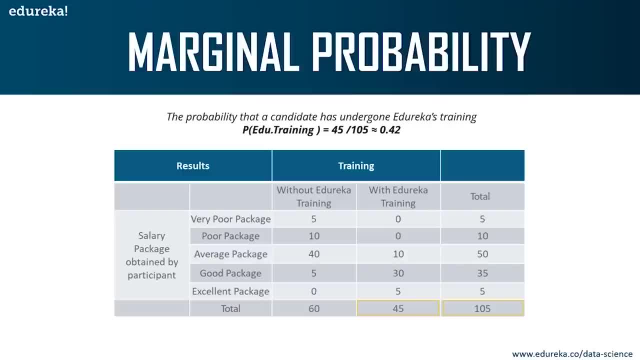 45.. 45 divided by 105, since 45 is the number of candidates with Edureka training and 105 is the total number of candidates, So you get a value of approximately 0.42.. All right, that's the probability of a candidate that has undergone Edureka's training. 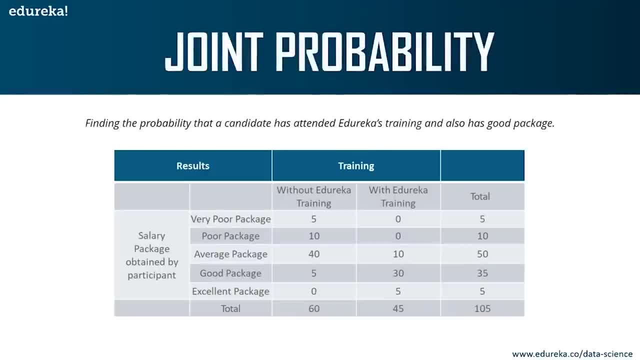 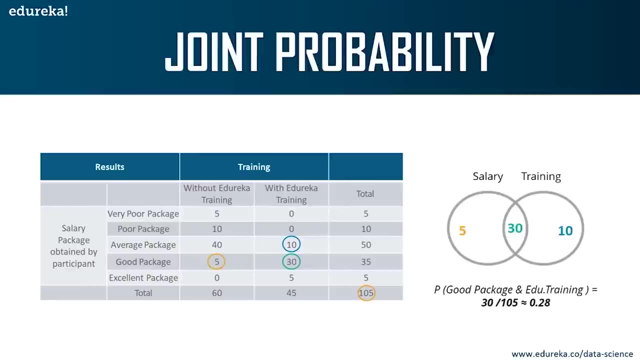 Next question: find the probability that a candidate has attended Edureka's training and also has good package. Now, this is obviously a joint probability problem, right? So how do you calculate this? Now, since our table is quite formatted, we can directly find that people who have gotten a good package, along with 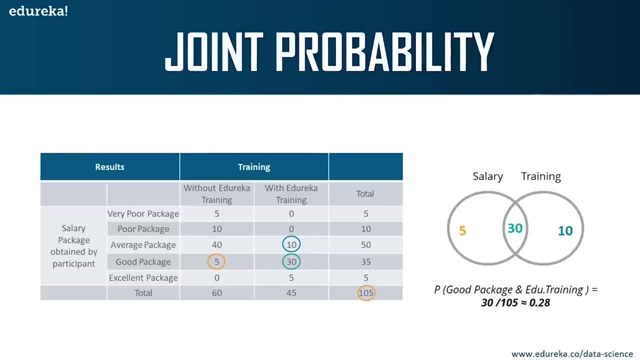 Edureka training are 30, right? So out of 105 people, 30 people have Edureka training and a good package, right? They specifically asking for people with Edureka training. Remember that, right? The question is: find the probability that a candidate has attended Edureka's. 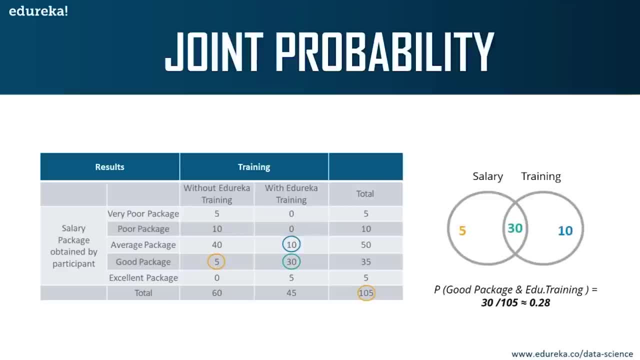 training and also has a good package, All right. so you need to consider two factors, that is, a candidate Who's attended Edureka's training and who has a good package. So clearly, that number is 30, 30 divided by total number of candidates. 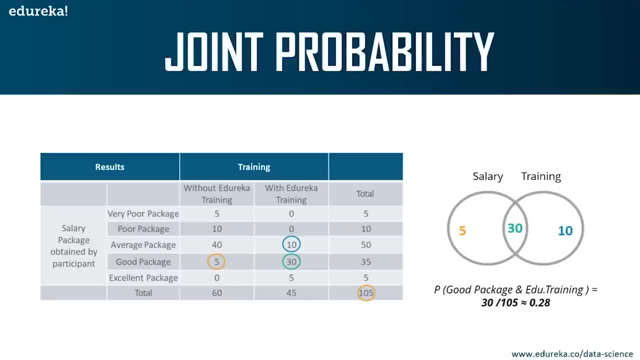 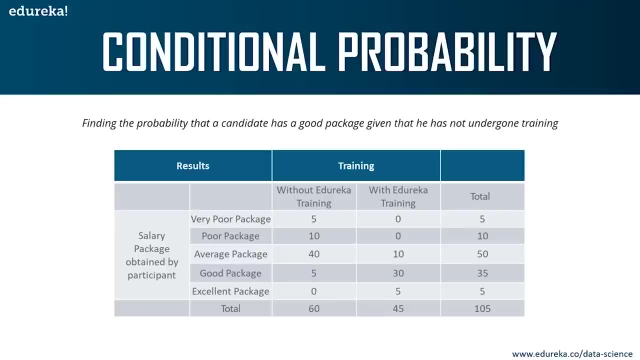 which is 105, right, So here you get the answer clearly. Next, we have find the probability that a candidate has a good package, given that he has not undergone training. Okay, Now, this is clearly conditional probability, because here you're defining a 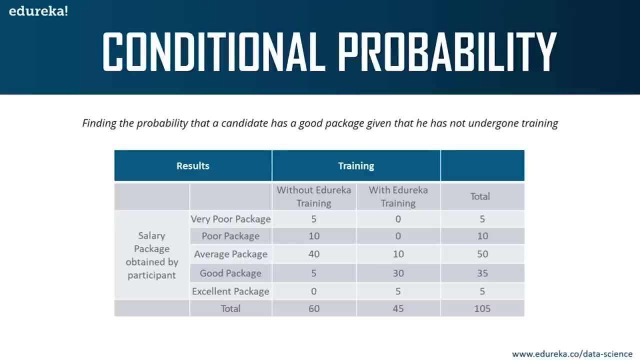 condition. You're saying that you want to find the probability of a candidate who has a good package, given that he's not undergone any training. right, The condition is that he's not undergone any training. All right. So the number of people who have not undergone training are 60 and out of 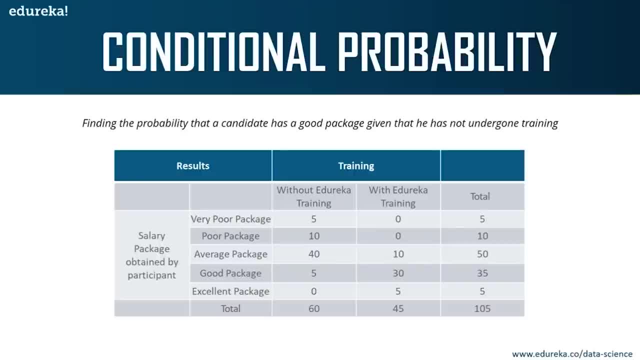 that five of them have got a good package right. So that's why this is 5 by 60 and not 5 by 105, because here they've clearly mentioned has a good package, given that he has not undergone training. So you have to only consider people who have not undergone training. 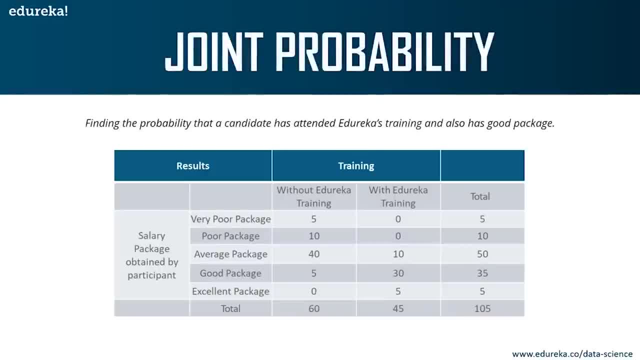 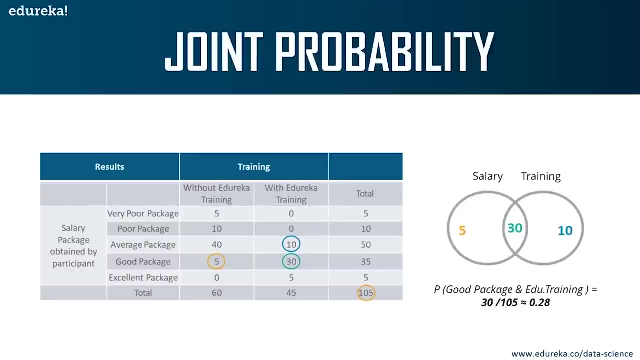 Next question: find the probability that a candidate has attended Edureka's training And also has good package. Now, this is obviously a joint probability problem, Right? So how do you calculate this? Now, since our table is quite formatted, we can directly find that people who have gotten a good package along with Edureka training are 30. 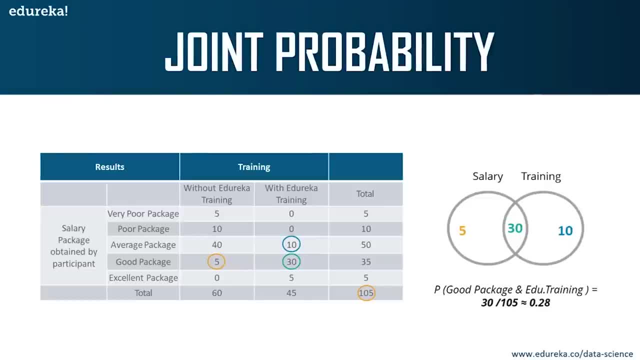 Right. So out of 105 people, 30 people have Edureka training and a good package, Right? They specifically asking for people with Edureka training. Remember that right. The question is: find the probability that a candidate has undergone Edureka's training. 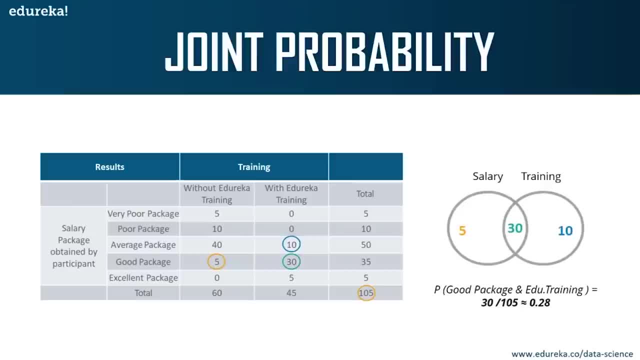 Right That a candidate has attended Edureka's training and also has a good package, All right. so you need to consider two factors: That is, a candidate who's attended Edureka's training and who has a good package. So clearly, that number is 30.. 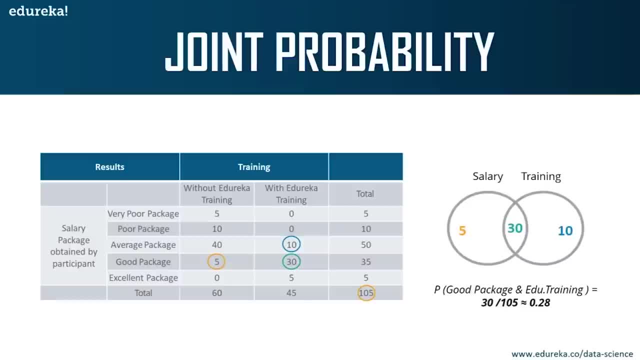 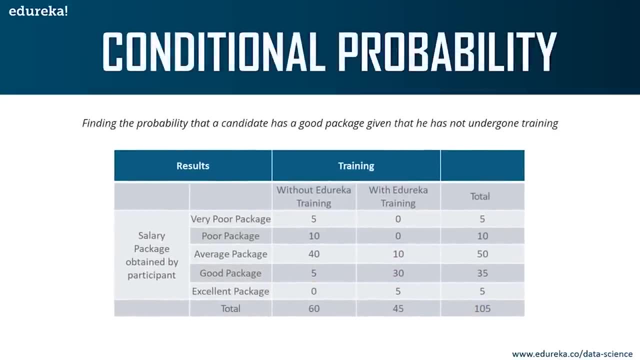 30 divided by total number of candidates, which is 105.. Right, So here you get the answer clearly. Next, we have find the probability that a candidate has a good package, given that he has not undergone training. Okay, Now, this is clearly conditional probability, because here you're defining a condition. 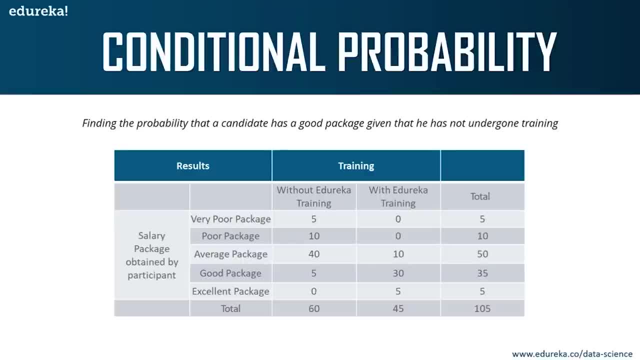 You're saying that you want to find the probability of a candidate who has a good package given that he's not undergone any training. Right, The condition is that he's not undergone any training, All right. So the number of people who have not undergone training are 60, and out of that, five of them have got a good package. 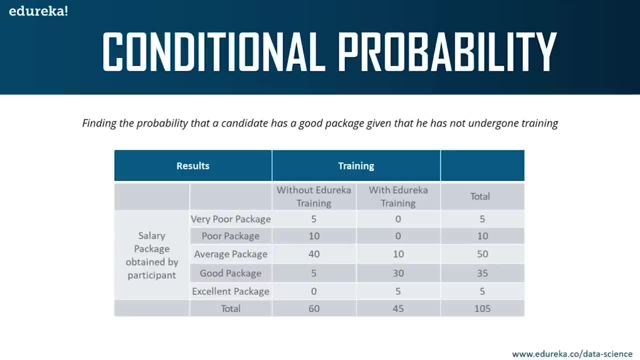 Right. So that's why this is 5 by 60 and not 5 by 105, because here they've clearly mentioned has a good package, given that he has not undergone training. So you have to only consider people who have not undergone training. 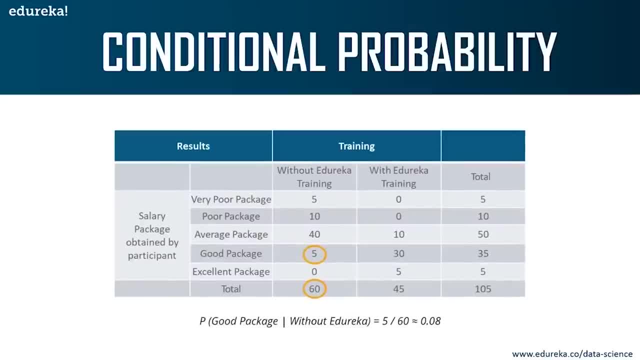 Right, So only five people who have not undergone training have gotten a good package, Right? So 5 divided by 60, you get a probability of around 0.08, which is pretty low, Right? Okay, So this was all about the different types of probability. 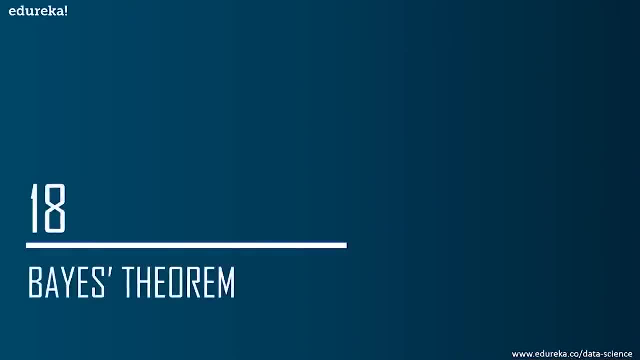 Now let's move on and look at our last topic in probability, which is Bayes Theorem. Now, guys, Bayes Theorem is a very important concept when it comes to statistics and probability. It is majorly used in naive bias algorithm. 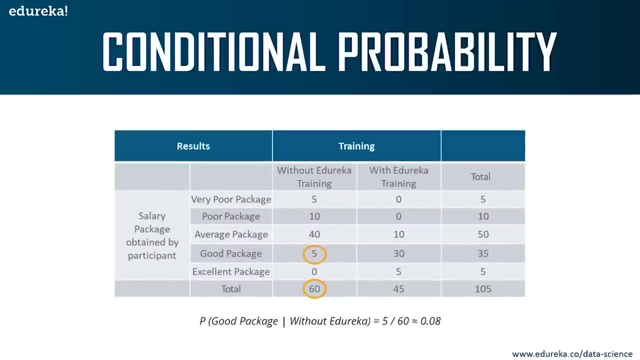 right? So only five people who have not undergone training have gotten a good package, right? So 5 divided by 60, you get a probability of around 0.08, which is pretty low, right? Okay, So this was all about the different types of probability. 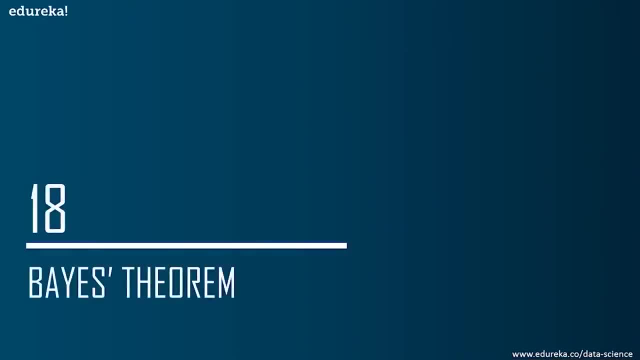 Now let's move on and look at our last topic in probability, which is Bayes theorem. Now, guys, Bayes theorem is a very important concept when it comes to statistics and probability. It is majorly used in naive bias algorithm. 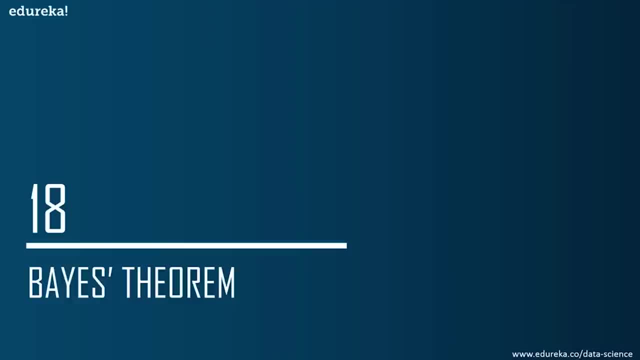 Those of you who aren't aware, naive bias is a supervised learning classification algorithm and it is mainly used in Gmail spam filtering right. A lot of you might have noticed that if you open up Gmail, you'll see that you have a folder called spam. 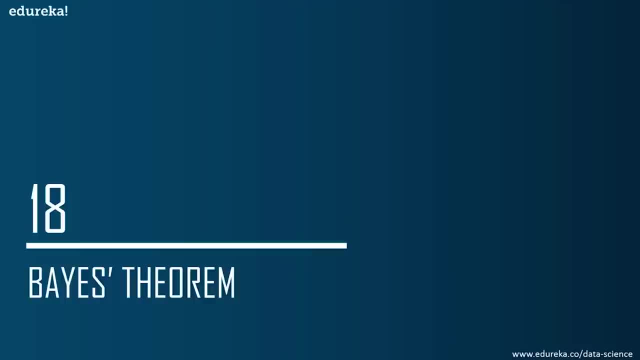 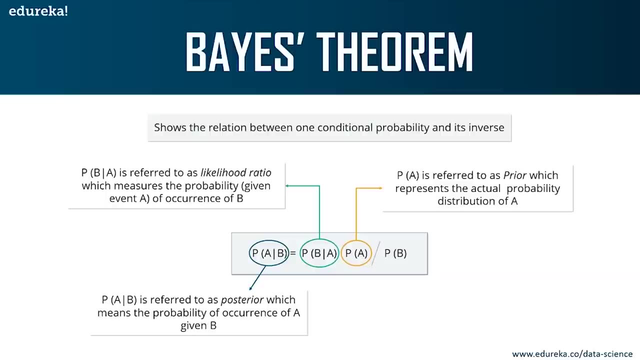 right. All of that is carried out through machine learning and the algorithm used. there is naive bias, right. So now let's discuss what exactly the Bayes theorem is and what it denotes. The Bayes theorem is used to show the relation between one conditional 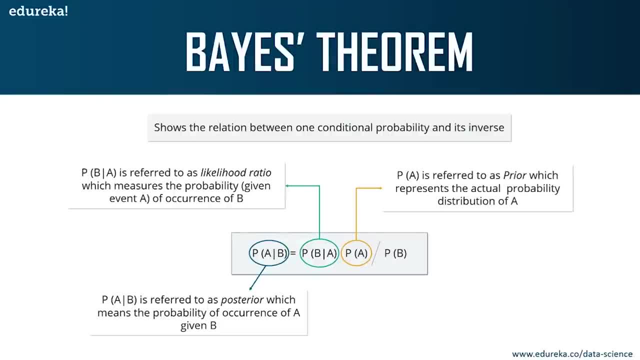 probability and its inverse. All right, basically, it's nothing but the probability of an event occurring, based on prior knowledge of conditions that might be related to the same event. Okay, So mathematically, the Bayes theorem is represented like this: 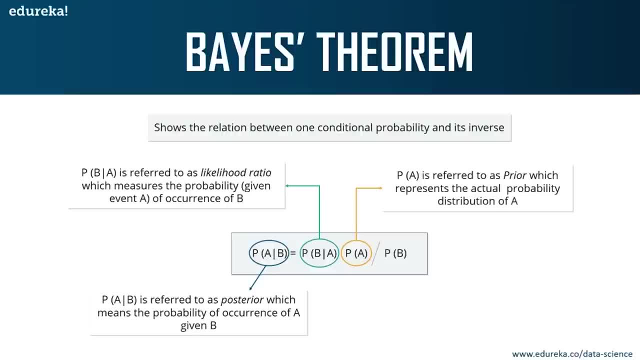 right, Like shown in this equation. the left-hand term is referred to as the likelihood ratio, which measures the probability of occurrence of event B, given an event A. Okay, on the left-hand side is what is known as the posterior. 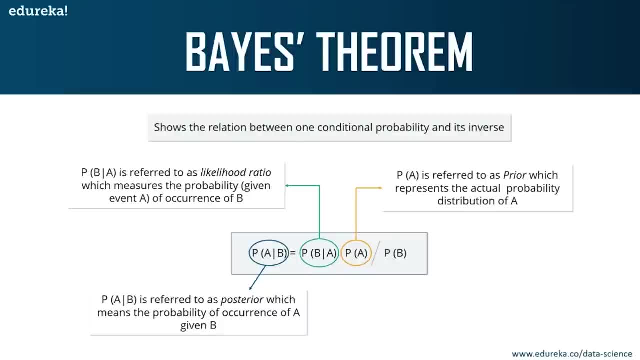 All right is referred to as posterior, which means that the probability of occurrence of A given an event B right. The second term is referred to as the likelihood ratio All right. this measures the probability of occurrence of B given an event A. 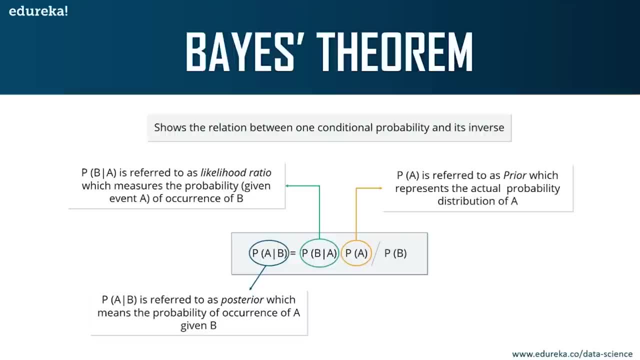 Now P of A is also known as the prior, which refers to the actual probability distribution of A, and P of B is again the probability of B right. This is the Bayes theorem. Now, in order to better understand the Bayes theorem, 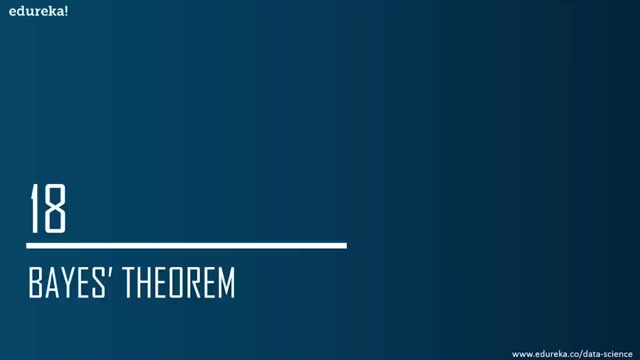 Those of you who aren't aware, naive bias is a supervised learning classification algorithm and it is mainly used in Gmail spam filtering Right. A lot of you might have noticed that if you open up Gmail, you'll see that you have a folder called spam. 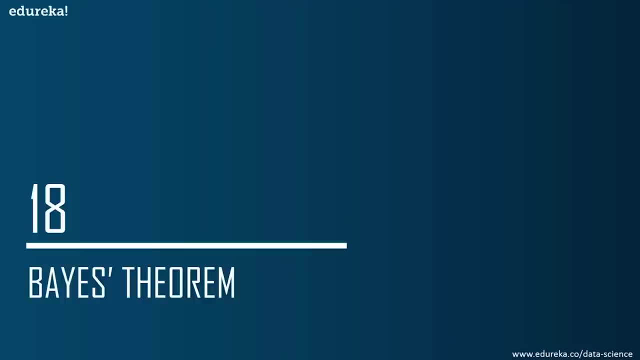 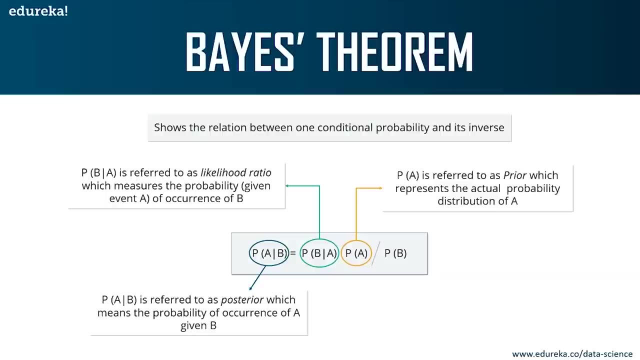 Right. All of that is carried out through machines. In learning and the algorithm used there is naive bias, Right. So now let's discuss what exactly the Bayes Theorem is and what it denotes. The Bayes Theorem is used to show the relation between one conditional probability and its inverse. 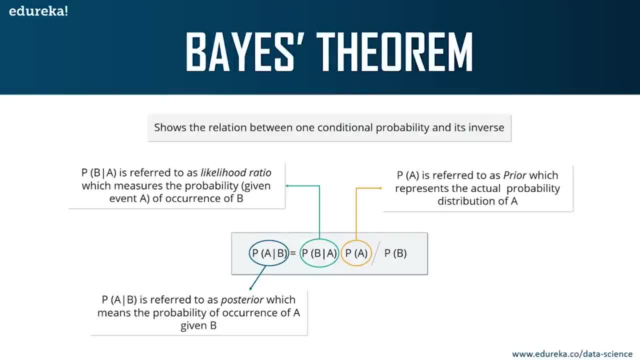 All right, basically, it's nothing but the probability of an event occurring, based on prior knowledge of conditions that might be related to the same event. Okay, so mathematically the Bayes Theorem is represented Like this right, like shown in this equation. 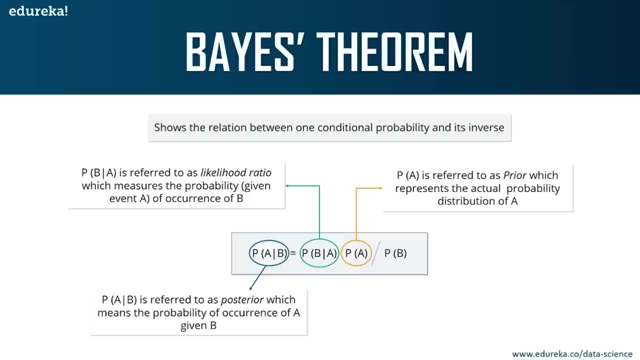 The left-hand term is referred to as the likelihood ratio, which measures the probability of occurrence of event B given an event A. okay, on the left hand side is what is known as the posterior. All right is referred to as posterior, which means that the probability of occurrence of a given an event B 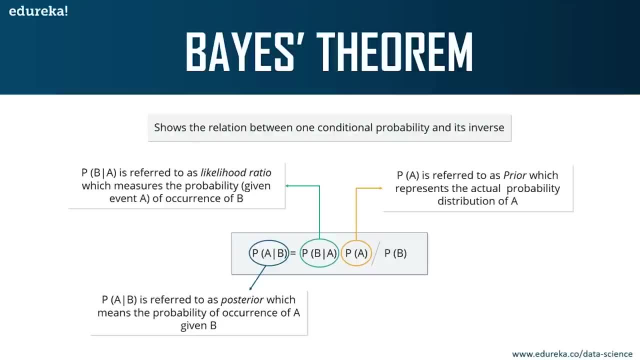 right. The second term is referred to as the likelihood ratio. All right. this measures the probability of occurrence of B Given an event A. now P of A is also known as the prior, which refers to the actual probability distribution of A, and P of B is again the probability of B. 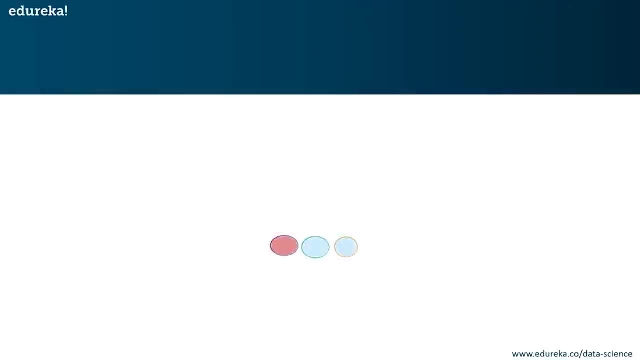 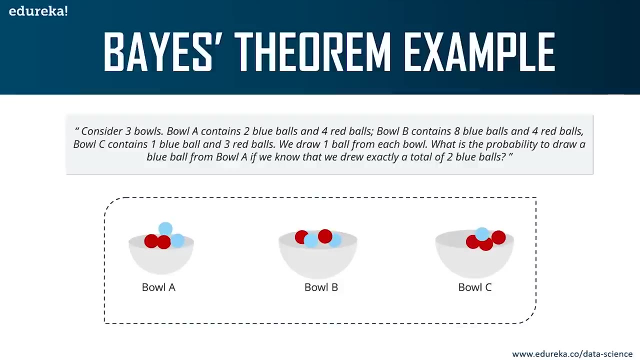 Right, This is the Bayes Theorem. Now, in order to better understand the Bayes Theorem, Let's look at a small example. Let's say that we have three bowels. We have bowel A, bowel B and bowel C. 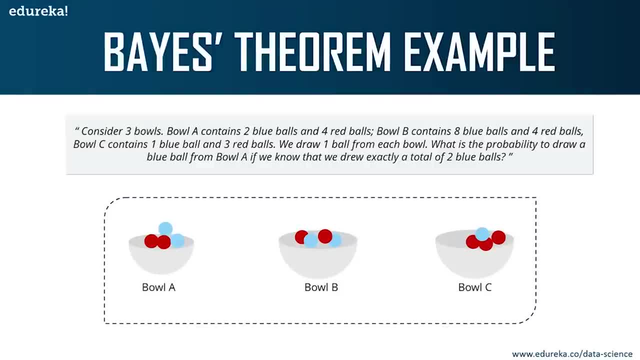 Okay, bowel A contains two blue balls and four red balls. Bowel B contains eight blue balls and four red balls. Bowel C contains one blue ball and three red balls. Now, if we draw one ball from each bowel, what is the probability to draw a blue ball from a bowel A? 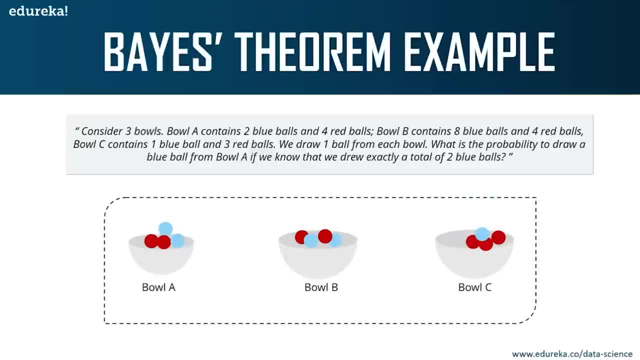 If we know that we drew exactly a total of two blue balls, right? If you didn't understand the question, please reread it. I shall pause for a second or two, Right? So I hope all of you have understood the question. 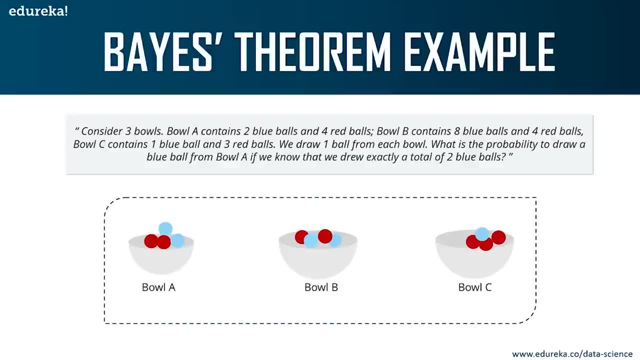 let's look at a small example. Let's say that we have three bowels. We have bowel A, bowel B and bowel C. Okay, bowel A contains two blue balls and four red balls. Bowel B contains eight blue balls and four red balls. 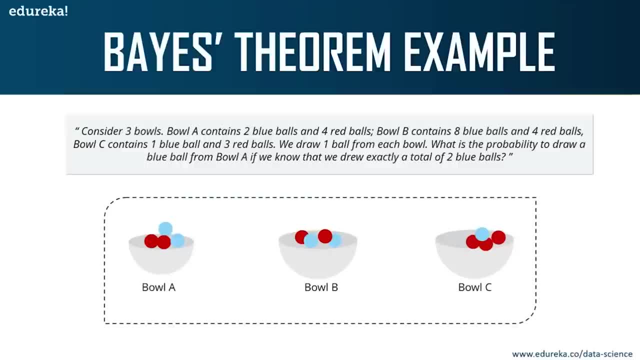 Bowel C contains one blue ball and three red balls. Now, if we draw one ball from each bowel, what is the probability to draw a blue ball from a bowel A If we know that we drew exactly a total of two blue balls? 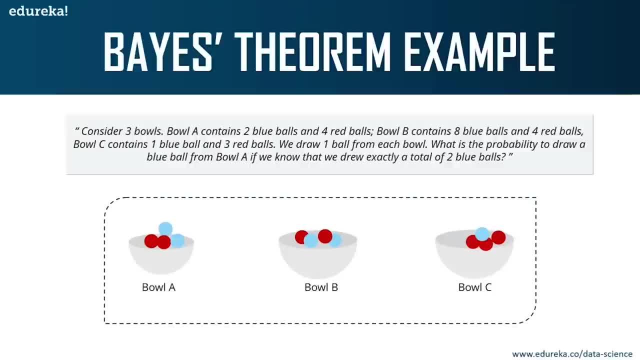 right, If you didn't understand the question, please reread it. I shall pause for a second or two, right? So I hope all of you have understood the question. Okay, Now, what I'm going to do is I'm going to draw a blueprint for you and tell you how exactly to solve the problem. 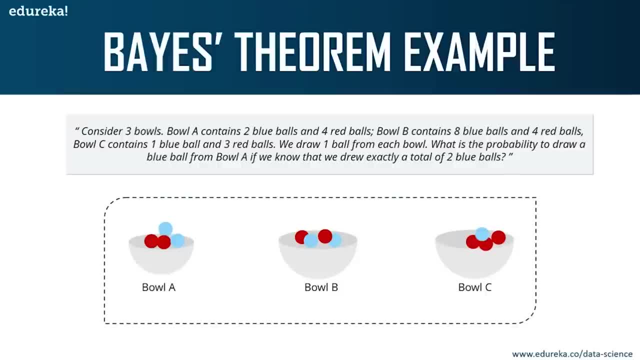 But I want you all to give me the solution to this problem. right, I'll draw a blueprint, I'll tell you what exactly the steps are, but I want you to come up with a solution on your own right. the formula is also given to you. everything is given to you, all you. 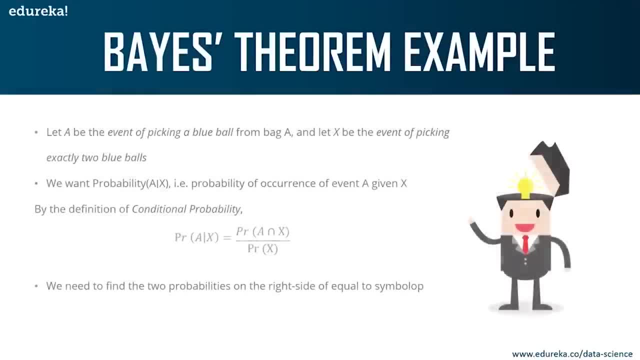 have to do is come up with a final answer. right, let's look at how you can solve this problem. so, first of all, what we'll do is let's consider a: all right, let a be the event of picking a blue ball from bag a and let x be the event of picking exactly two blue balls. right, because these are the. 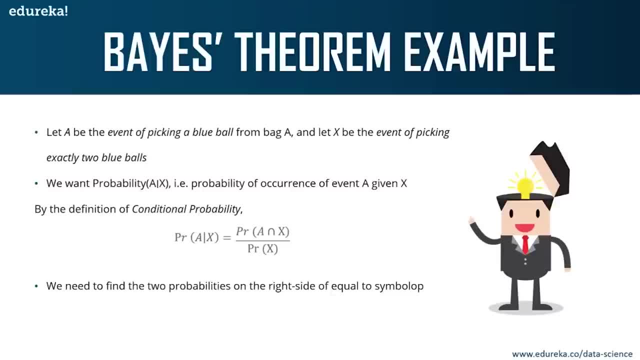 two events that we need to calculate the probability of now. there are two probabilities that you need to consider here. one is the event of picking a blue ball from bag a and the other is the event of picking exactly two blue balls. okay, so these two are represented by a and x. 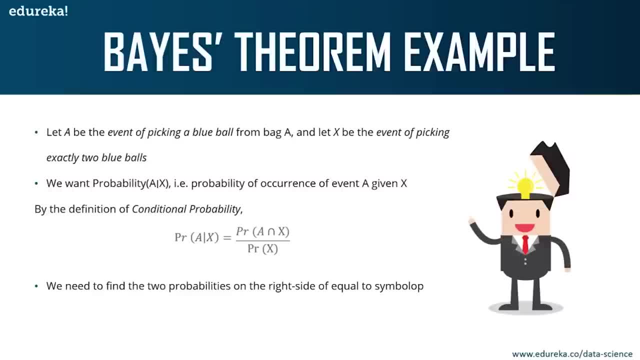 respectively. so what we want is the probability of occurrence of event a given x, which means that, given that we're picking exactly two blue balls, what is the probability that we are picking a blue ball from bag a? so, by the definition of conditional probability, this is exactly what our equation will look like, correct? this is basically occurrence of event a. 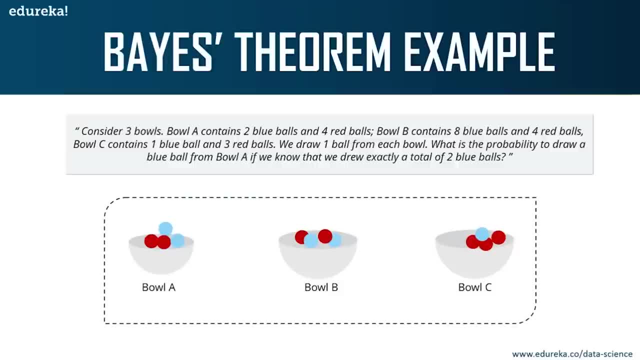 Okay, Now what I'm going to do is I'm going to draw a blueprint for you and tell you how exactly to solve the problem. but I want you all to give me the solution to this problem. Right, I'll draw a blueprint. 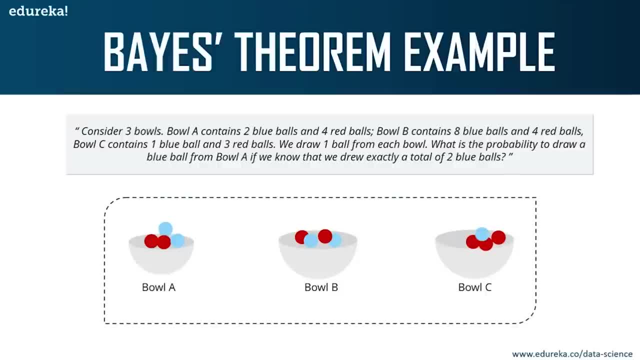 I'll tell you what exactly the steps are, but I want you to come up with a solution on your own Right. The formula is also given to you. Everything is given to you. All you have to do is come up with a final answer. 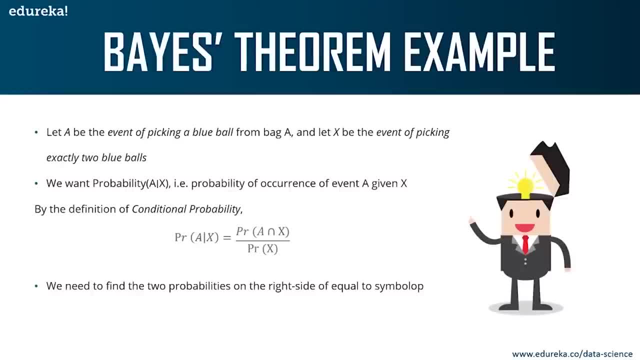 Right, Let's look at how you can solve this problem. So, first of all, what we'll do is: let's consider A. All right, let A be the event of picking a blue ball from bag A, And let X be the event of picking exactly two blue balls. 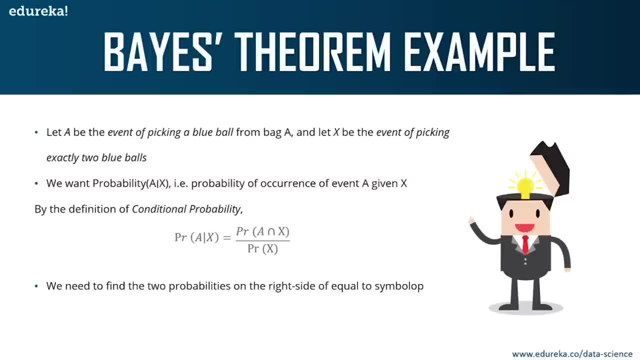 Right, Because these are the two events that we need to calculate the probability of Now. there are two probabilities that you need to consider here. One is the event of picking a blue ball from bag A, And the other is the event of picking exactly two blue balls. 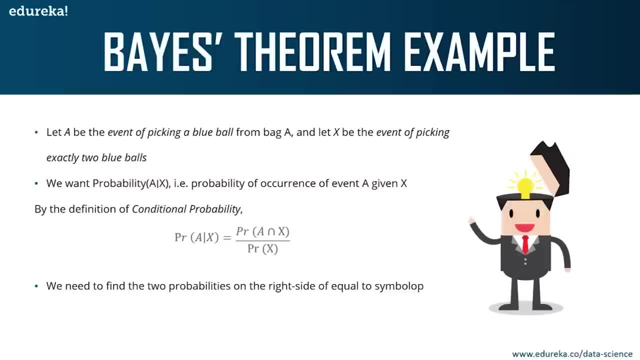 Okay, So these two are represented by A and X respectively. So what we want is the probability of occurrence of event A given X, which means that, given that we're picking exactly two blue balls, What is the probability that we are picking a blue ball from bag A? 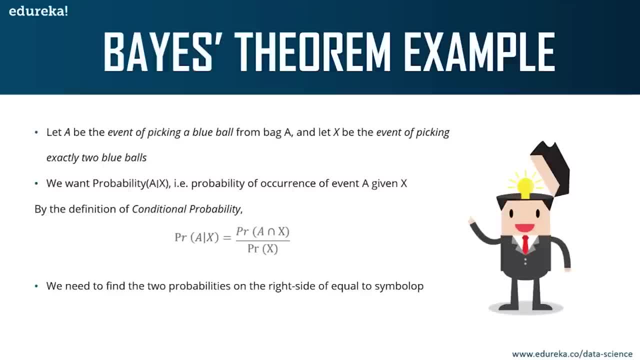 So, by the definition of conditional probability, this is exactly what our equation will look like, Correct. This is basically occurrence of event A given an event X, And this is the probability of A and X, And this is the probability of X alone. 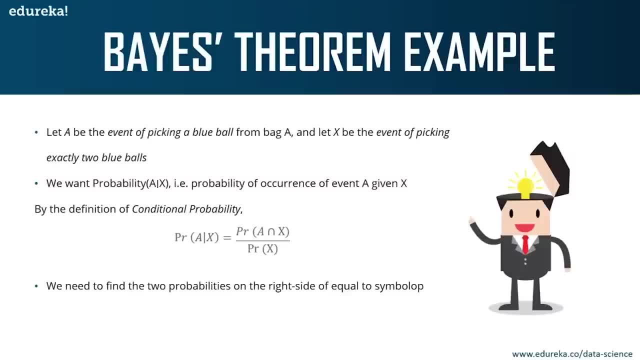 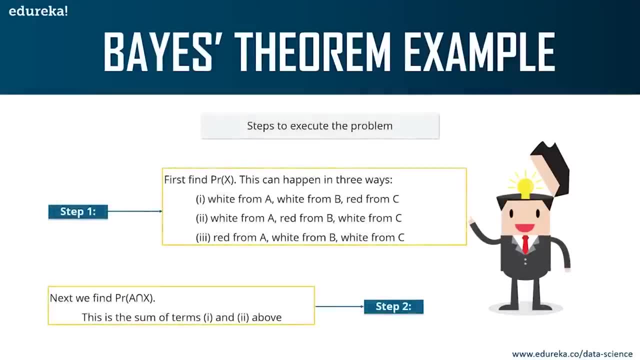 Correct. Now what we need to do is we need to find these two probabilities, which is probability of A and X occurring together and probability of X. Okay, This is the entire solution. So how do you find the probability of X? This you can do in three ways. 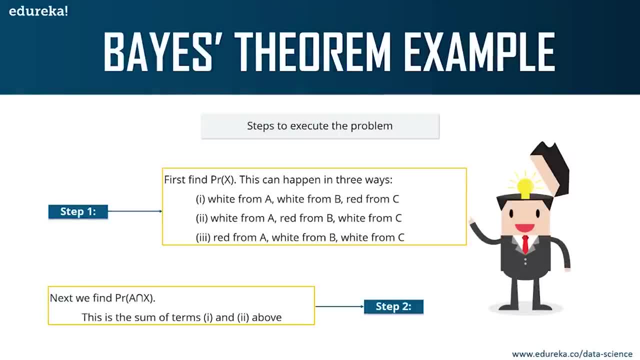 So first is white ball from A, either white from B or red from C. Now, first is to find the probability of X. X basically represents the event of picking exactly two blue balls, Right? So these are the three ways in which it is possible. 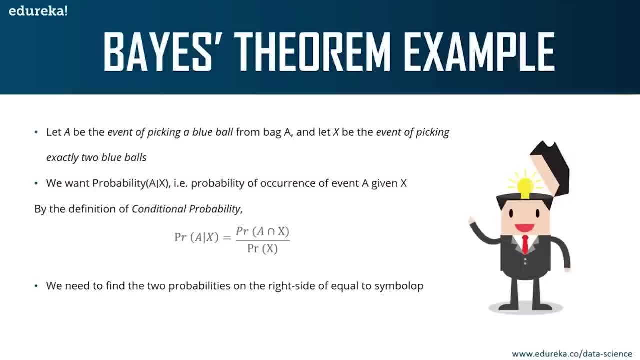 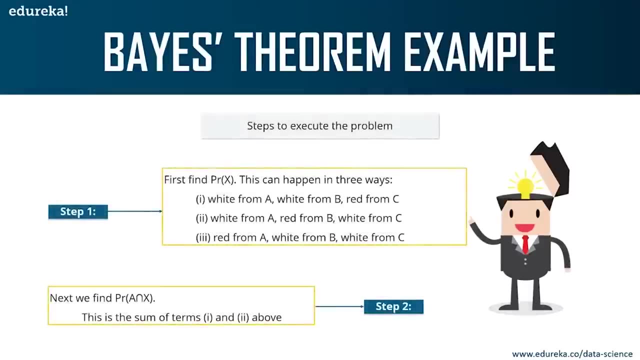 given an event, x, and this is the probability of a and x, and this is the probability of x alone, correct? now what we need to do is we need to find these two probabilities, which is probability of a and x occurring together and probability of x. okay, this is the entire solution. 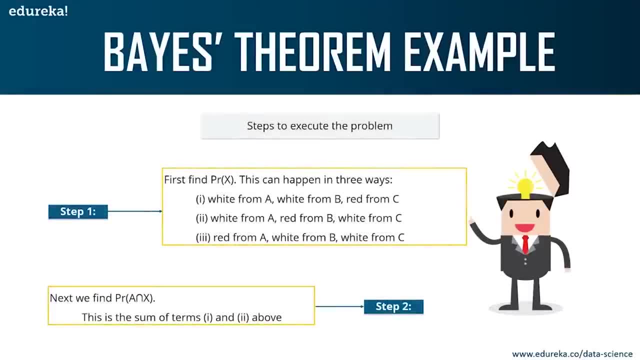 so how do you find p probability of x? this you can do in three ways. so first is white ball from a, either white from b or red from c. now, first is to find the probability of x. x basically represents the event of picking exactly two blue balls, right? so these are the 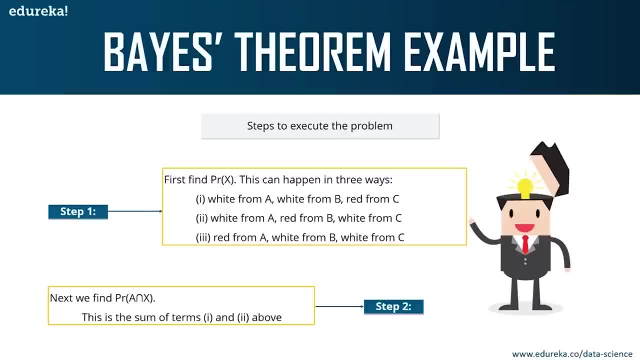 three ways in which it is possible. so you will pick one blue ball from bowel a and one from bowel b. in the second case, you can pick one from a and another blue ball from c. in the third case, you can pick a blue ball from bag b and a blue ball. 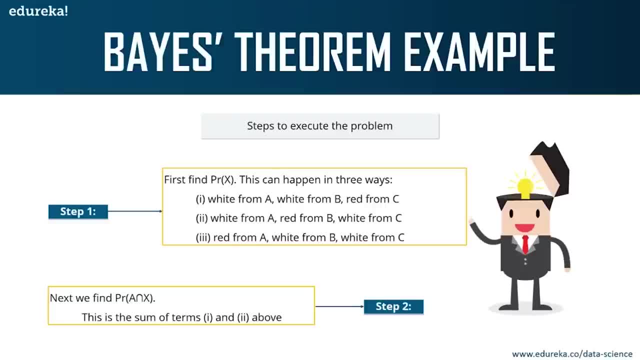 from bag c? right, these are the three ways in which it is possible, so you need to find the probability of each of this. step two is that you need to find the probability of a and x occurring together. this is the sum of terms one and two. okay, this is because in both of these events, you're picking. 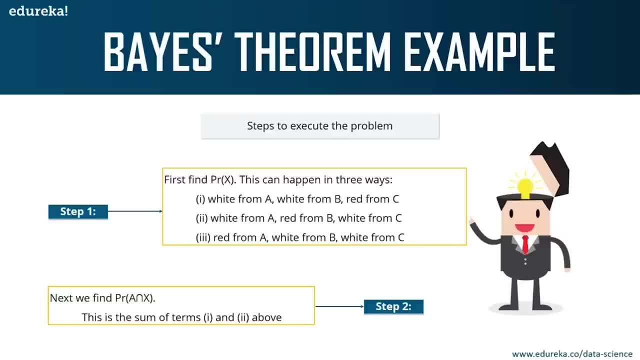 a ball from bag a correct. so guys find out this probability and let me know in the comment section your answer in the comment section. all right, we'll see if you get the answer right. i gave you the entire solution to this. all you have to do is substitute the value, right? if you want a second? 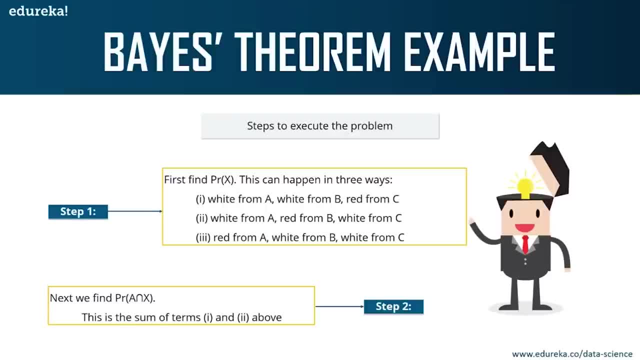 or two. i'm going to pause on the screen so that you can go through this in a more clearer way. right, remember that you need to calculate two probabilities. the first probability that you need to calculate is the event of picking a blue ball from bag a, given that you're picking exactly two. 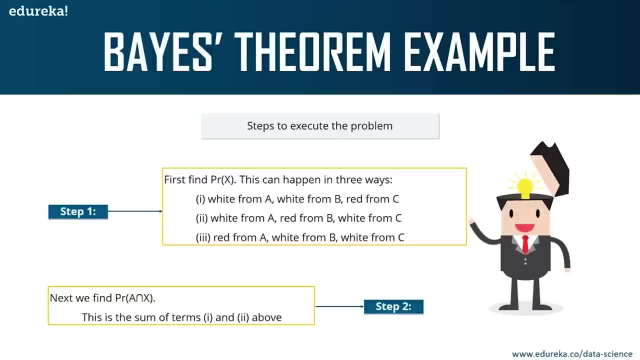 blue balls. okay, she's also going to fit for this. however, the second probability you need to calculate is the event of picking exactly two blue balls. all right, these are the two probabilities you need to calculate. so remember that and this is the solution, all right. so, guys, make sure you mention. 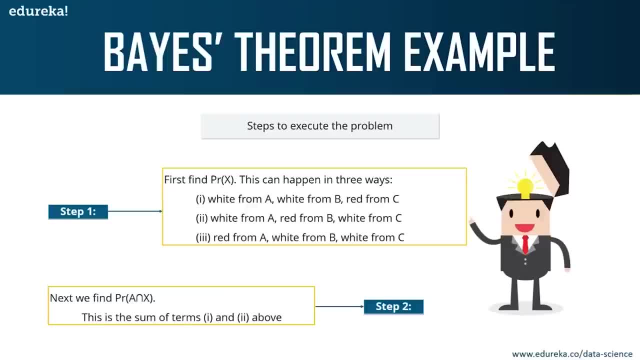 So you'll pick one blue ball from bowel A and one from bowel B. In the second case, you can pick one from A and another blue ball from C. In the third case, you can pick a blue ball from bag B and a blue ball from bag C. 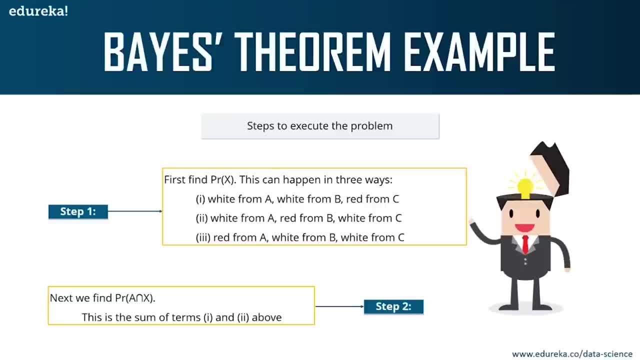 Right, These are the three ways in which it is possible, So you need to find the probability of each of this. Step two is that you need to find the probability of A and X occurring together. This is the sum of terms one and two. 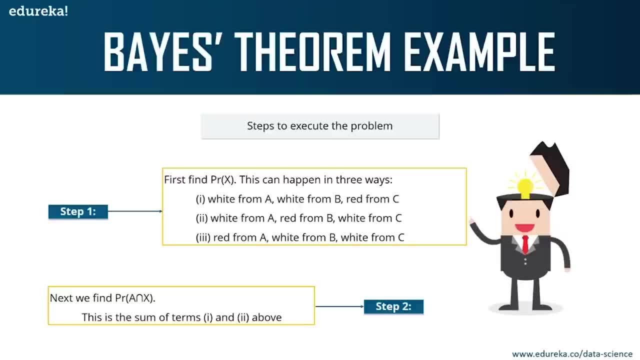 Okay, This is because in both of these events you're picking a ball from bag A, Correct. So guys, find out this probability and let me know your answer in the comment section. All right, We'll see if you get the answer. 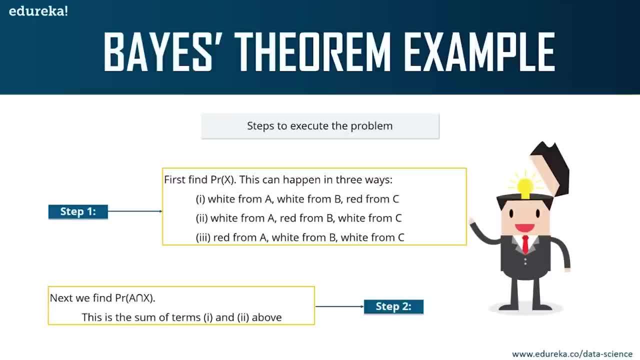 Right. I gave you the entire solution to this. All you have to do is substitute the value, Right. If you want a second or two, I'm going to pause on the screen so that you can go through this in a more clearer way. 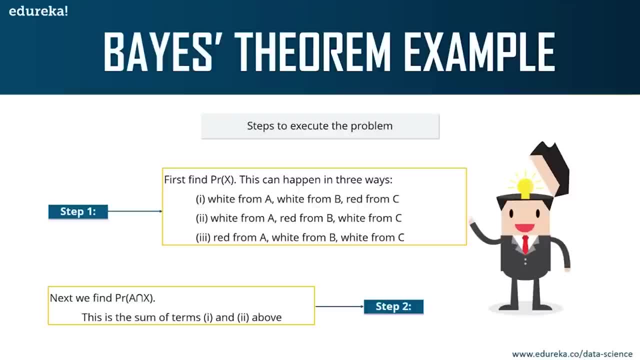 Right, Remember that you need to calculate two probabilities. The first probability that you need to calculate is the event of picking a blue ball from bag A. given that you're picking exactly two blue balls, Okay. The second probability you need to calculate is the event of picking exactly. 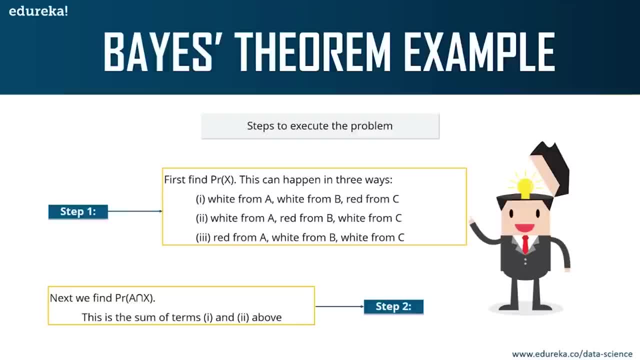 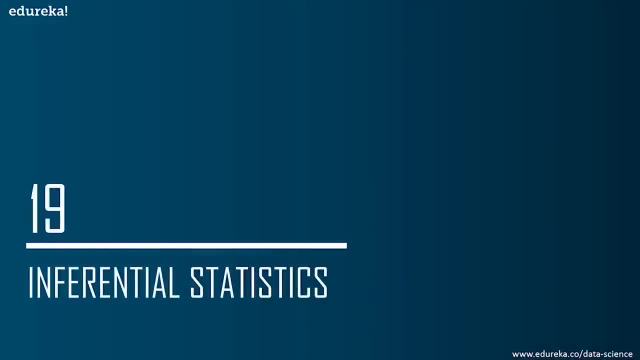 two blue balls. All right, These are the two probabilities you need to calculate, So remember that and this is the solution, All right? So, guys, make sure you mention your answers in the comment section. for now, Let's move on and look at our next topic, which is the inferential statistic. 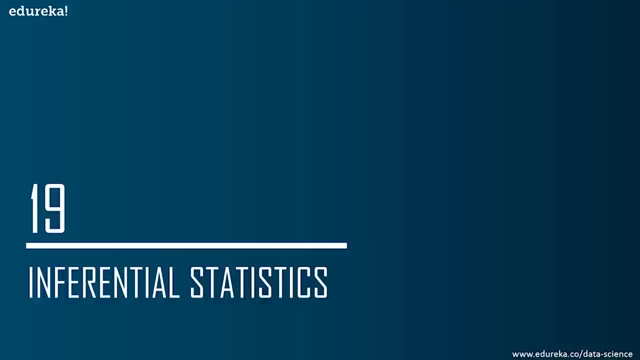 So, guys, we just completed the probability module. right now We'll discuss inferential statistics, which is the second type of statistics. We discussed descriptive statistics earlier. All right, So, like I mentioned earlier, inferential statistics, also known as statistical inference, is a branch of statistics that deals with forming inferences and 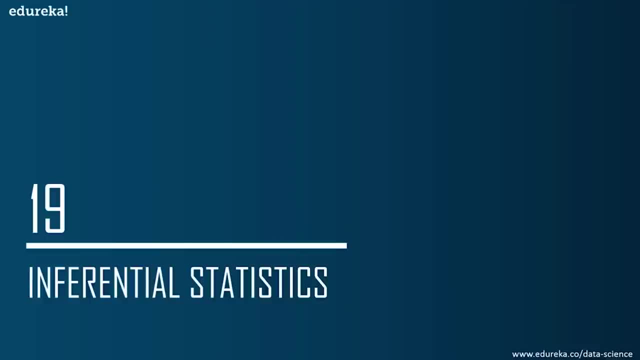 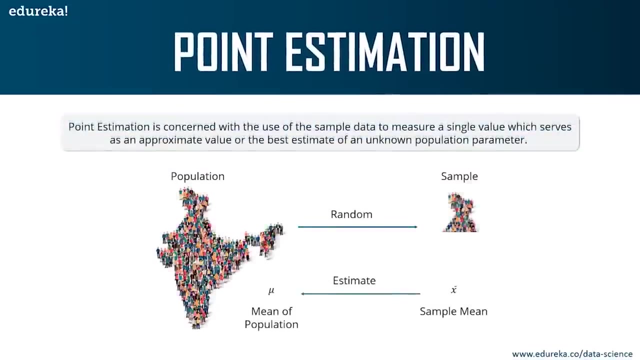 predictions about a population based on a sample of data taken from the population. All right, and the question you should ask Is: how does one form inferences or predictions on a sample? The answer is: you use point estimation. Okay, Now you must be wondering: what is point estimation? one estimation is concerned. 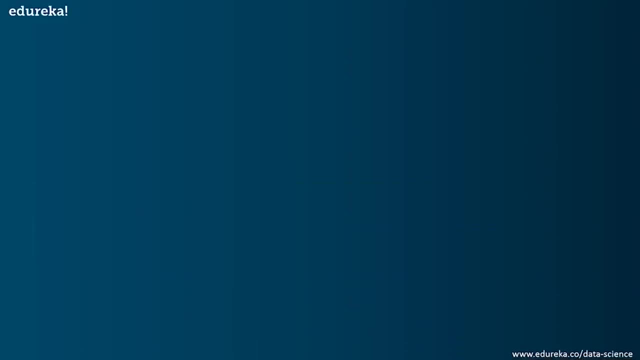 your answers in the comment section. for now, let's move on and look at our next topic, which is the inferential statistics. so, guys, we just completed the probability module. right now we'll discuss inferential statistics, the second type of statistics. we discussed descriptive statistics earlier, all right, so 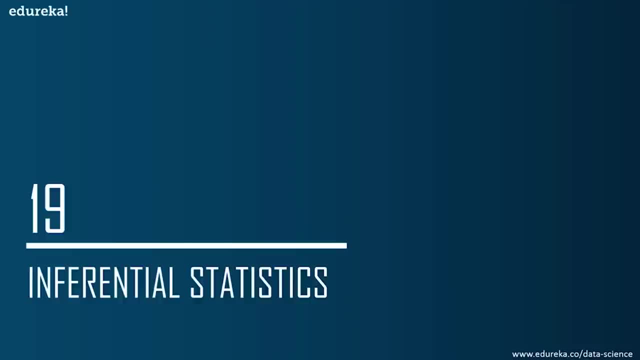 like i mentioned earlier, inferential statistics, also known as statistical inference, is a branch of statistics that deals with forming inferences and predictions about a population based on a sample of data taken from the population. all right, and the question you should ask is: how does one form inferences or predictions on a sample? the answer is: you use point estimation. okay, now you. 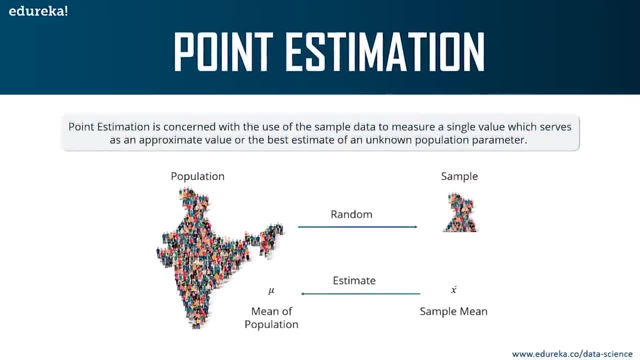 must be wondering: what is point estimation point? estimation is concerned with the use of the sample data to measure a single value which serves as an approximate value or the best estimate of an unknown population parameter. that's a little confusing. let me break it down to you, for example. 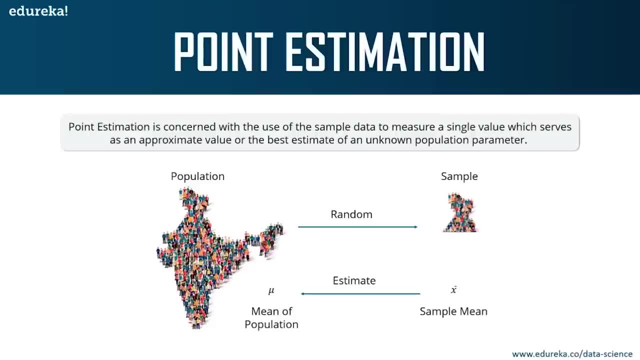 in order to calculate the mean of a huge population. what we do is we calculate the mean of a huge population. what we do is we calculate the mean of a population, is we first draw out the sample of the population and then we find the sample mean. right, the sample. 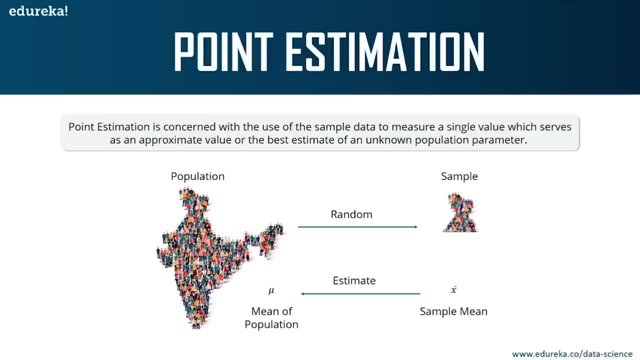 mean is then used to estimate the population mean. this is basically point estimate. you're estimating the value of one of the parameters of the population, right? basically the mean. you're trying to estimate the value of the mean. this is what point. estimation is the two main terms in point. 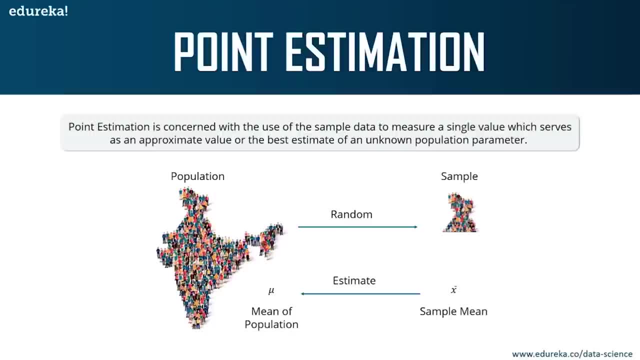 estimation, or there's something known as the estimator, and the estimate estimator is a function of the sample that is used to find out the estimate. All right, in this example it's basically the sample mean, right? So a function that calculates the sample mean. 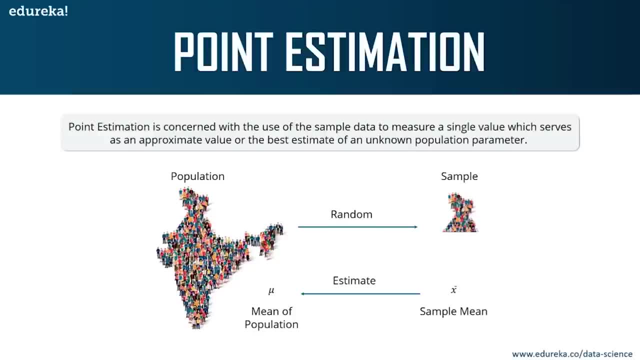 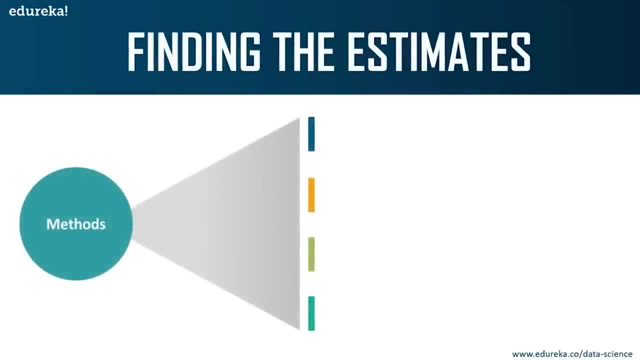 is known as the estimator, And the realized value of the estimator is the estimate Right. so I hope point estimation is clear. Now how do you find the estimates? There are four common ways in which you can do this. The first one is method of moments. 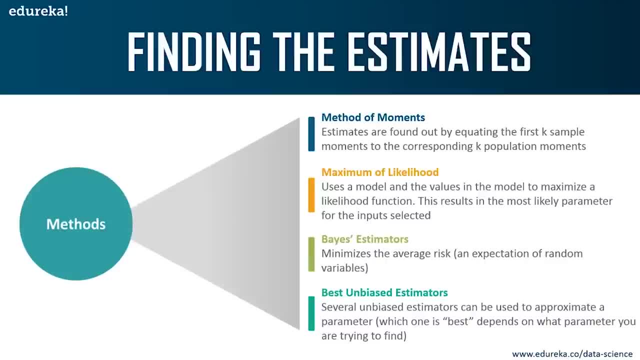 Here. what you do is you form an equation in the sample data set and then you analyze a similar equation in the population data set as well, Like the population, mean, population variance and so on. So, in simple terms, what you're doing is: 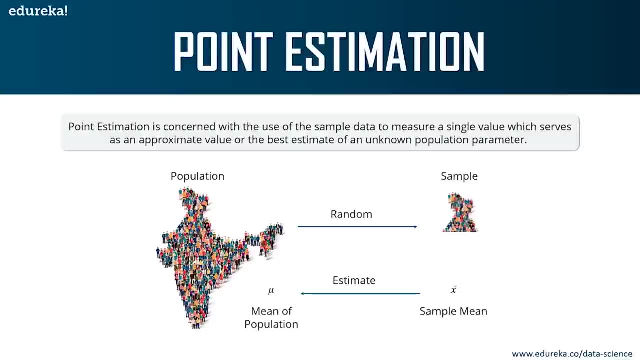 with the use of the sample data to measure a single value which serves as an approximate value or the best estimate of an unknown population parameter. That's a little confusing. Let me break it down to you. For example, in order to calculate the mean of a huge population, 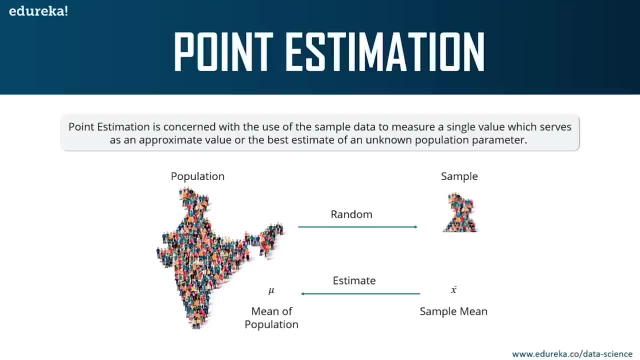 What we do is we first draw out the sample of the population and then we find the sample mean right. the sample mean is then used to estimate the population mean. this is basically point: estimate- your estimating the value of one of the parameters of the population right, basically the mean you're. 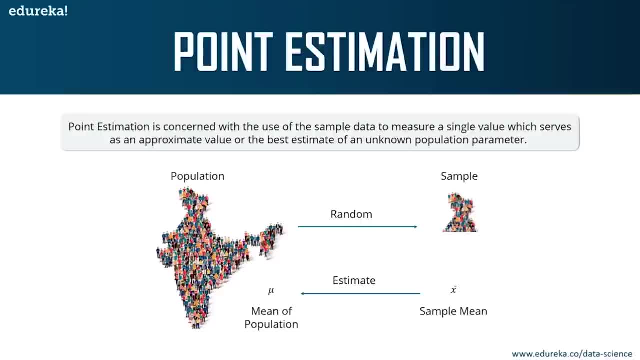 trying to estimate the value of the mean. this is what point. estimation is the two main terms in point: estimation, or there's something known as the estimator and there's something known as the estimate. estimator is a function of the sample that is used to find out the estimate. right in this example. 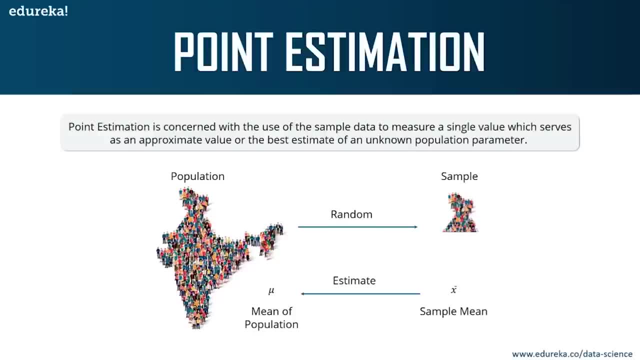 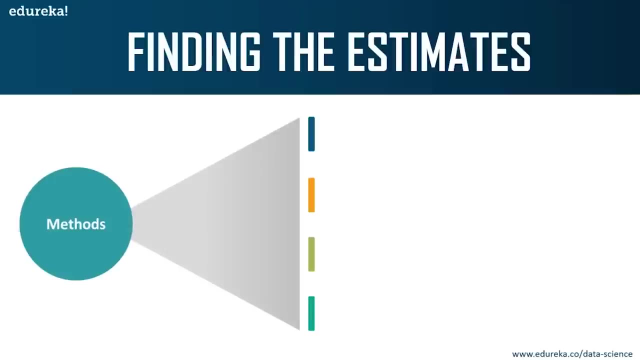 It's basically the sample mean, right? so a function that calculates a sample mean is known as the estimator, and the realized value of the estimator is the estimate, right? So I hope point estimation is clear. Now, how do you find the estimates? There are four common ways in which you can do this. 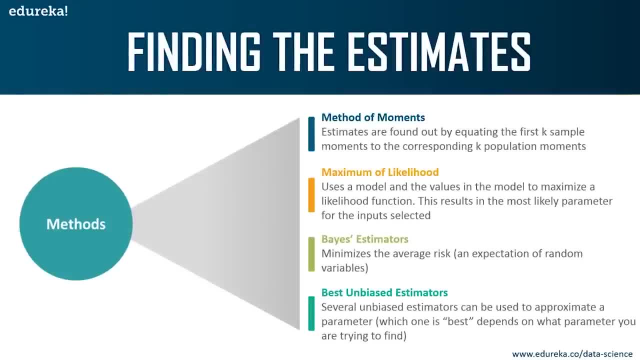 The first one is method of moments. here What you do is you form an equation in the sample, In the sample data set, and then you analyze a similar equation in the population data set as well, like the population, mean, population variance and so on. So, in simple terms, what you're doing is you're taking down some known facts about the population. 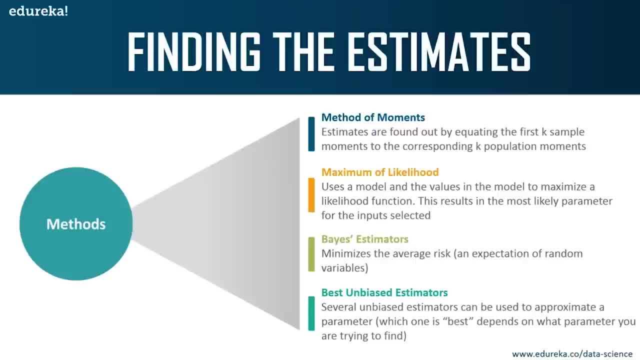 and you're extending those ideas to the sample. All right, once you do that, you can analyze the sample and estimate more essential or more complex values. right next We have maximum of likelihood of. this method basically uses a model to estimate A value. 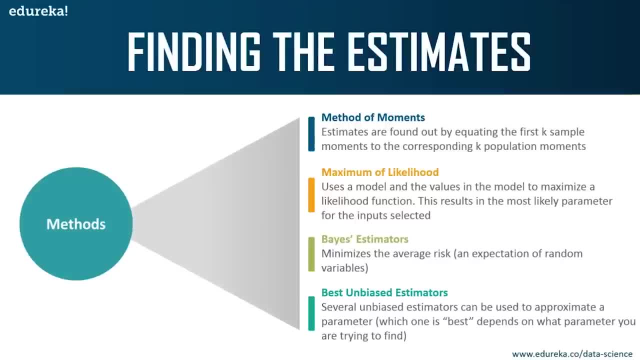 All right Now. a maximum likelihood is a majorly based on probability. So there's a lot of probability involved in this method. Next we have the base estimator. This works by minimizing the errors or the average risk. Okay, the base estimator has a lot to do with the Bayes theorem. 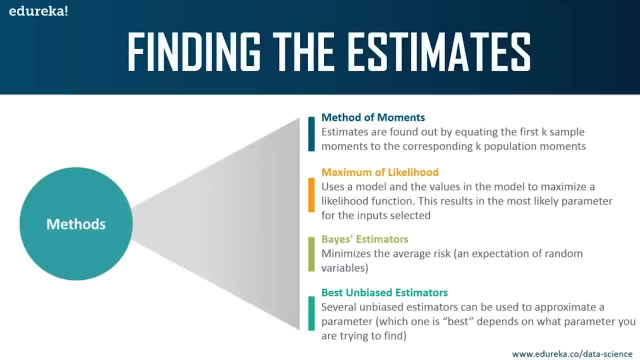 All right, let's not get into the depth of these estimation methods. Finally, we have the best unbiased estimators in this method. There are several unbiased estimators that can be used to appropriate, approximate a parameter. Okay, So, guys, these were a couple of methods that are used to find the estimate. 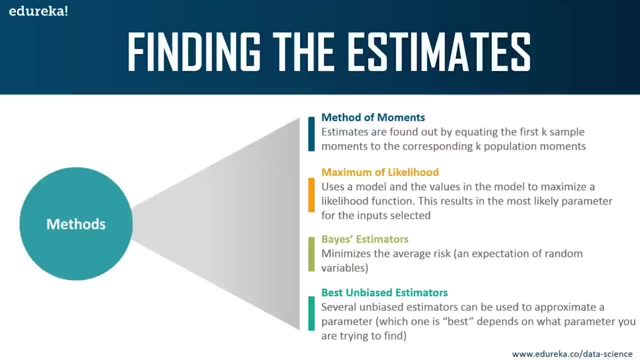 you're taking down some known facts about the population and you're extending those ideas to the sample. All right, once you do that, you can analyze the sample and estimate more essential or more complex values, right. Next we have maximum of likelihood. 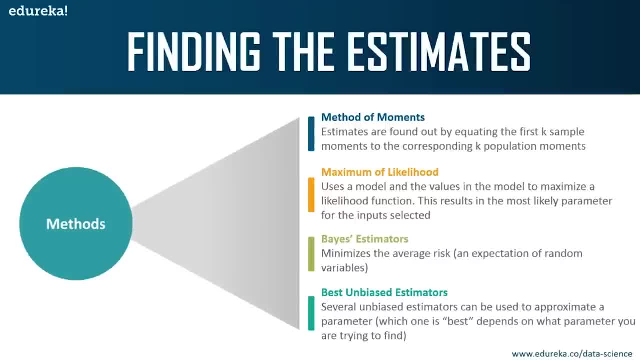 Now, this method basically uses a model to estimate a value. all right, Now, maximum of likelihood is majorly based on probability, so there's a lot of probability involved in this method. Next, we have the base estimator. This works by minimizing the errors or the average risks. 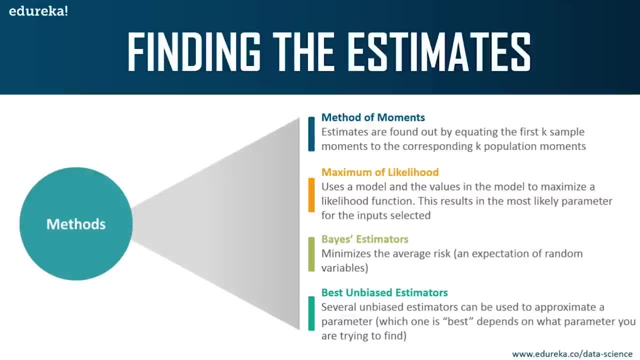 Okay, the base estimator has a lot to do with the bias theorem. all right, Let's not get into the depth of these estimation methods. Finally, we have the best unbiased estimators In this method. there are several unbiased estimators that can be used. 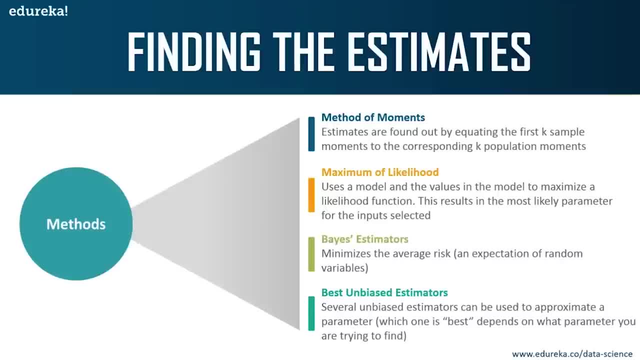 to approximate a parameter. okay, So, guys, these were a couple of methods that are used to find the estimate, but the most well-known method to find the estimate is known as the interval estimation. Okay, this is one of the most important estimation methods. 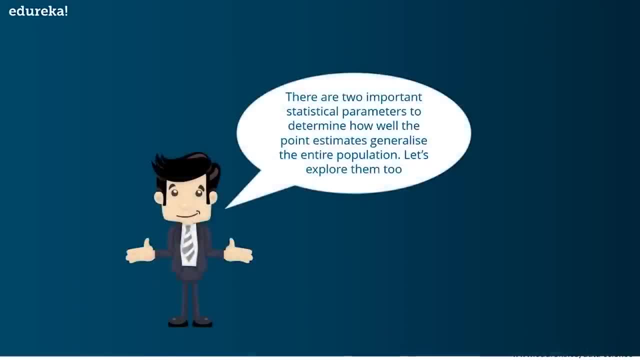 All right, this is where confidence interval also comes into the picture. right Apart from interval estimation, we also have something known as margin of error, So I'll be discussing all of this in the upcoming slides. So first let's understand what is interval estimate? okay, 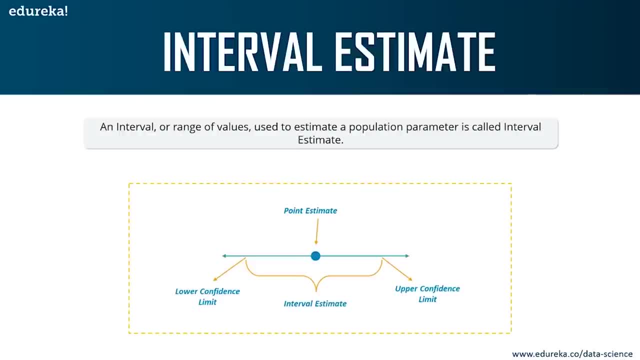 An interval or range of values which are used to estimate a population parameter is known as an interval estimation. Now, that's very understandable. Basically, what they're trying to say is: you're going to estimate the value of a parameter. Let's say you're trying to find the mean of a population. 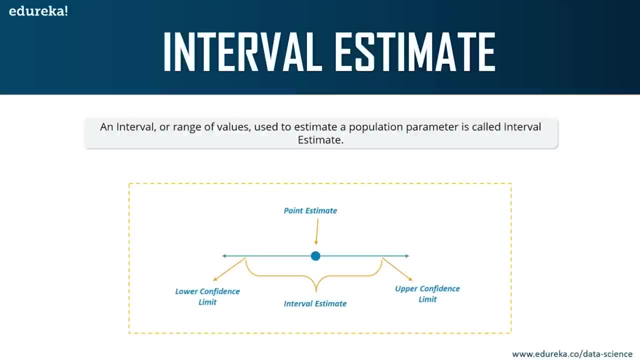 What you're going to do is you're going to build a range and your value will lie in that range or in that interval. All right, so this way your output is gonna be more accurate, Because you've not predicted a point estimation. 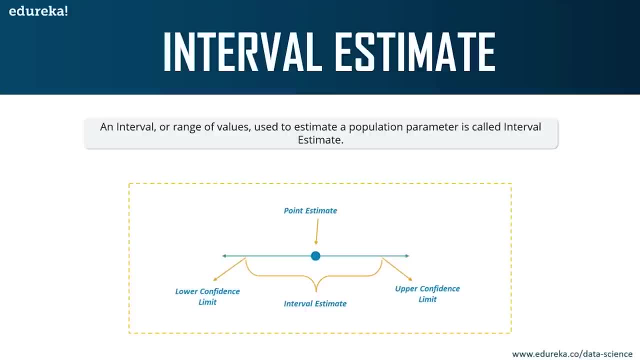 Instead, you have estimated an interval within which your value might occur. right, Okay, now this image clearly shows how point estimate and interval estimate are different. So, as interval estimate is obviously more accurate because you're not just focusing on a particular value, 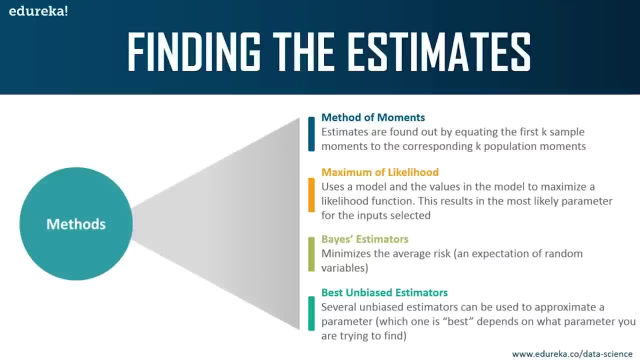 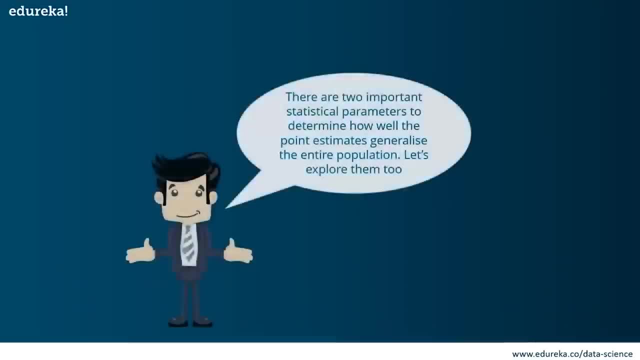 but the most well-known method to find the estimate is known as the interval estimation. Okay, This is one of the most important estimation methods. All right, This is where confidence interval also comes into the picture, Right. apart from interval estimation, We also have something known as margin of error. 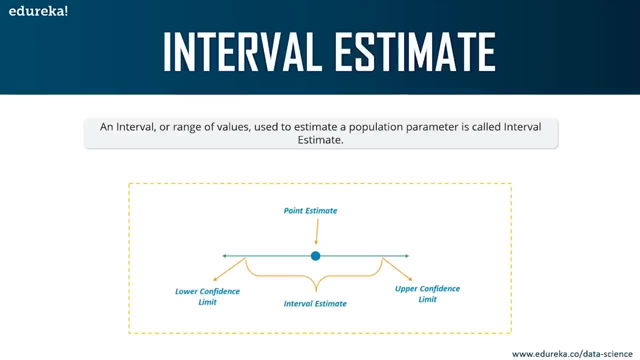 So I'll be discussing all of this in the upcoming slides. So first let's understand What is interval estimate. Okay, an interval or range of values which are used to estimate a population parameter is known as an interval estimation. right, That's very understandable. 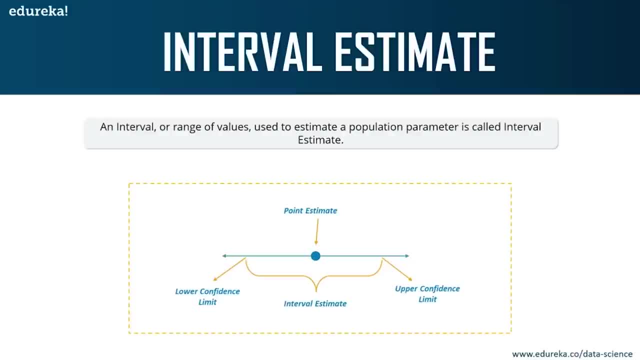 Basically, what they're trying to see is you're going to estimate the value of a parameter. Let's say you're trying to find the mean of a population. What you're going to do is you're going to build a range and your value will lie in that range or in that. 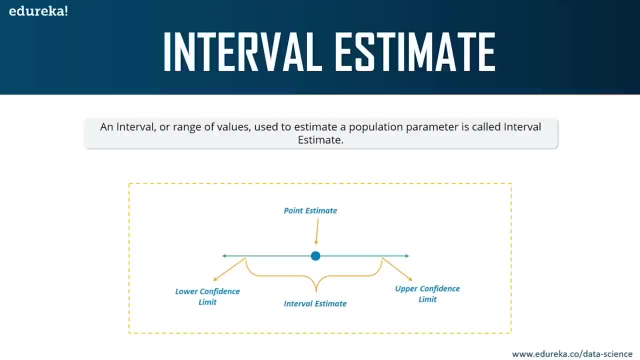 interval. All right. So this way, your output is going to be more accurate, Because you've not predicted a point estimation. Instead, You have estimated an interval within which your value might occur. Right, Okay, Now this image clearly shows how point estimate and interval estimate are different. 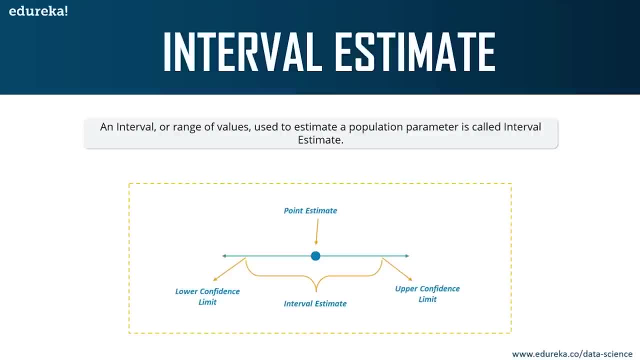 So, as interval estimate is obviously more accurate, because you're not just focusing on a particular value or a particular point in order to predict the probability. instead, you're saying that the value might be within this range between the lower confidence limit and the upper confidence limit. 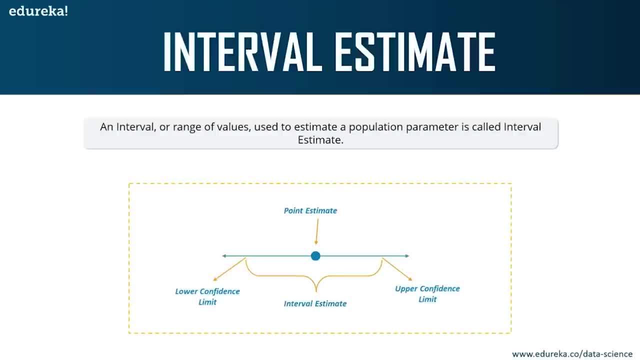 All right, this just denotes the range or the interval. Okay, if you're still confused about interval estimation, let me give you a small example. If I stated that I will take 30 minutes to reach the theater, This is known as point estimation. 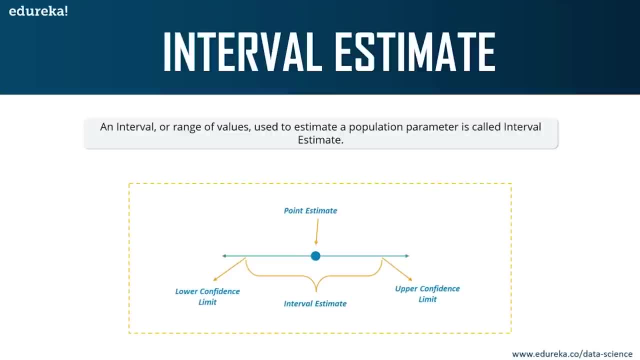 Okay, but if I stated that I will take between 45 minutes to an hour to reach the theater? This is an example of interval estimation. All right, I hope it's clear now. Now, interval estimation gives rise to two important statistical terminologies. 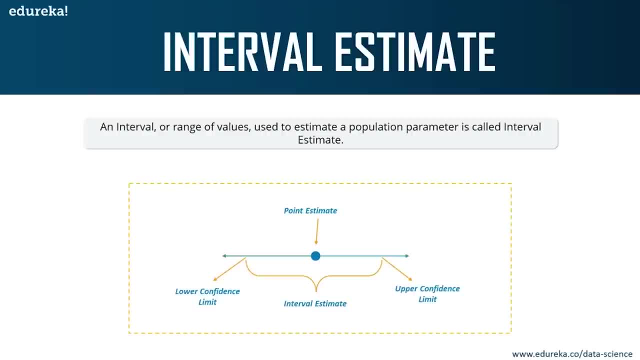 One is known as confidence interval and the other is known as margin of error. All right, So, guys, it's important that you pay attention to both of these terminologies. Confidence interval is one of the most significant measures that are used to check how essential a 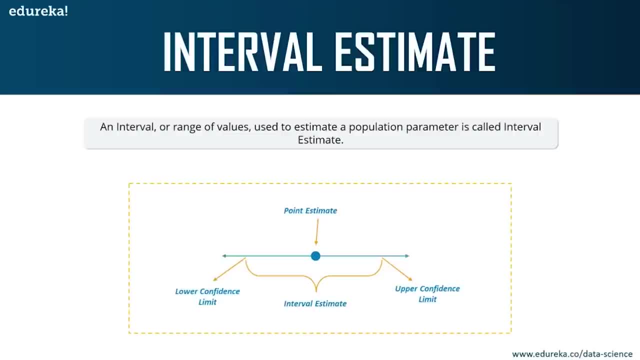 or a particular point in order to predict the probability. Instead, you're saying that the value might be within this range between the lower confidence limit and the upper confidence limit. all right, This just denotes the range or the interval. Okay, if you're still confused about interval estimation. 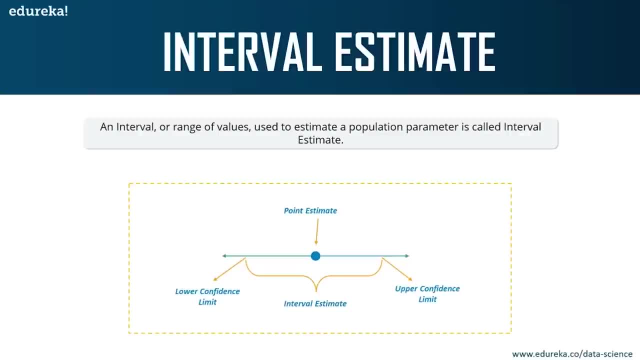 let me give you a small example. If I stated that I will take 30 minutes to reach the theater- this is known as point estimation- okay, But if I stated that I will take between 45 minutes to an hour to reach the theater? 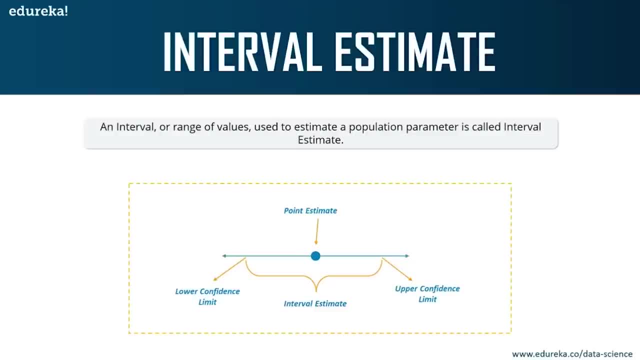 this is an example of interval estimation. all right, I hope it's clear now. Now, interval estimation gives rise to two important statistical terminologies. One is known as confidence interval and the other is known as margin of error. all right, 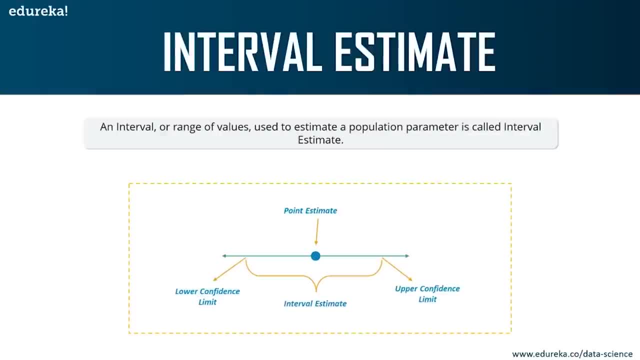 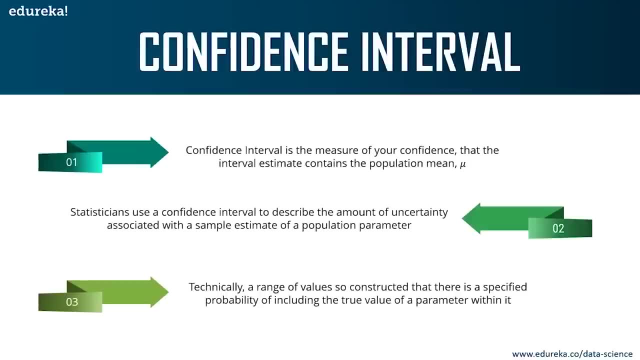 So, guys, it's important that you pay attention to both of these terminologies. Confidence interval is one of the most significant measures that are used to check how essential a machine learning model is. all right. So what is confidence interval? Confidence interval is the measure of your confidence. 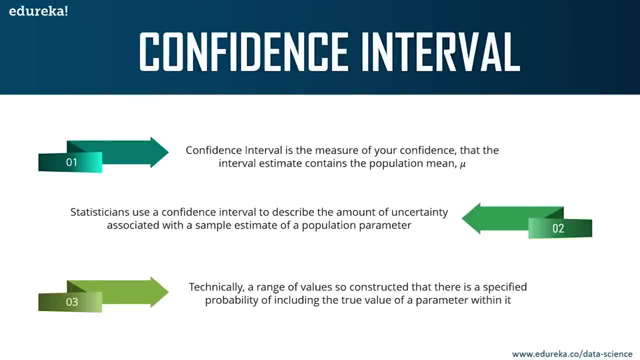 that the interval estimated contains the population parameter or the population mean or any of those parameters. right Now, statisticians use confidence interval to describe the amount of uncertainty associated with a sample estimate of a population parameter. Now, guys, this is a lot of definition. 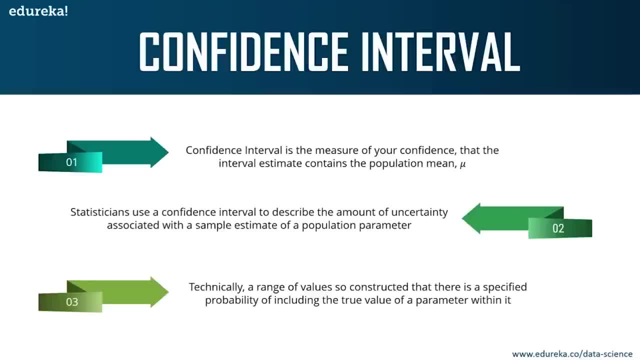 Let me just make you understand confidence interval with a small example. Okay, let's say that you perform a survey and you survey a group of cat owners to see how many cans of cat food they purchase in one year. okay, You test your statistics at the 99% confidence level. 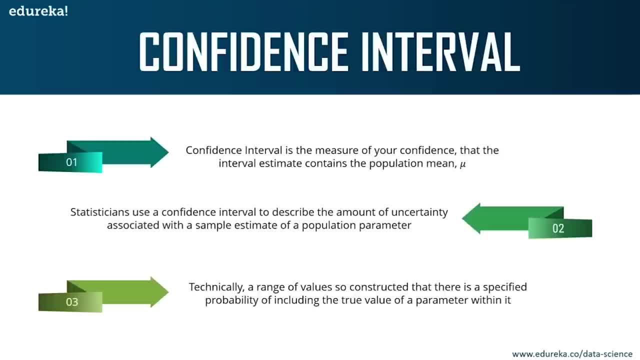 and you get a confidence interval of 100, 200.. This means that you think that the cat owners buy between 100 to 200 cans in a year And also, since the confidence level is 99%, it shows that you're very confident. 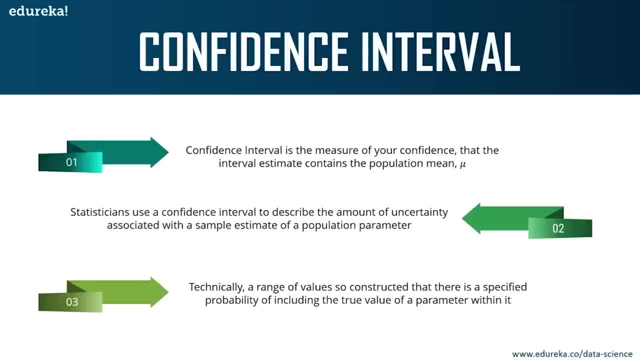 that the results are correct. okay, I hope all of you are clear with that. All right, so your confidence interval here will be 100, and 200, and your confidence level will be 99%. right, That's the difference between confidence interval. 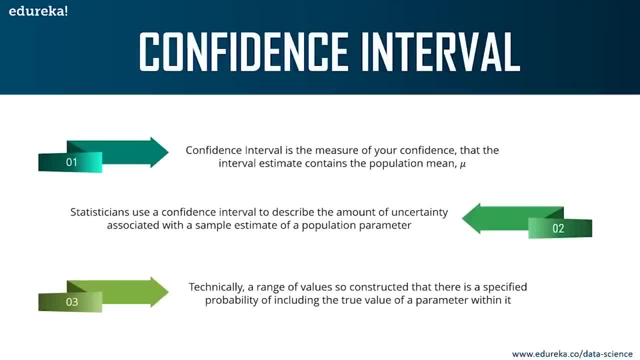 machine learning model is All right. So what is confidence interval? confidence interval is the measure of your confidence that the interval estimated contains the population parameter or the population mean or any of those parameters. Right now, statisticians use confidence interval to describe the amount of uncertainty associated. 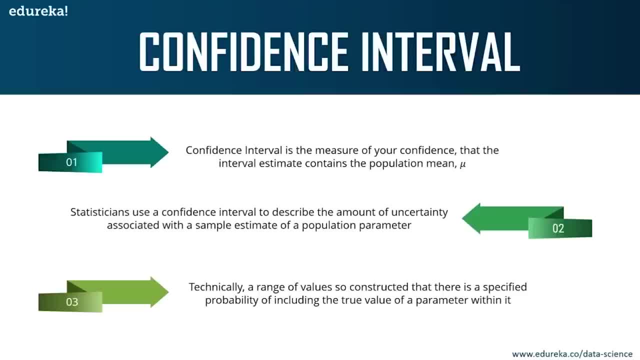 with the sample estimate of a population parameter. Now, guys, this is a lot of definition. Let me just make you understand confidence interval with a small example. Okay, let's say that you perform a survey and you survey a group of cat owners to see how many cans of cat food. 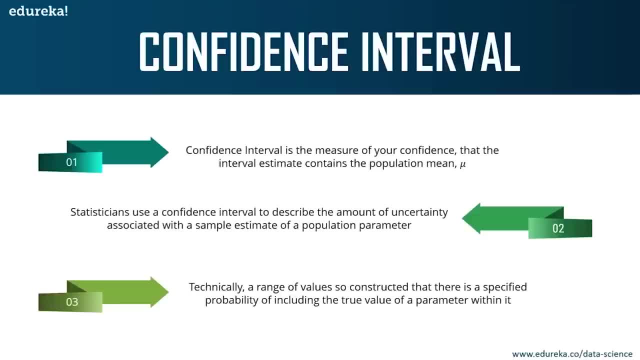 They purchase in one year. Okay, you test your statistics at the 99% confidence level and you get a confidence interval of hundred comma 200.. This means that you think that the cat owners by between 100 to 200 cans in a year and also since the 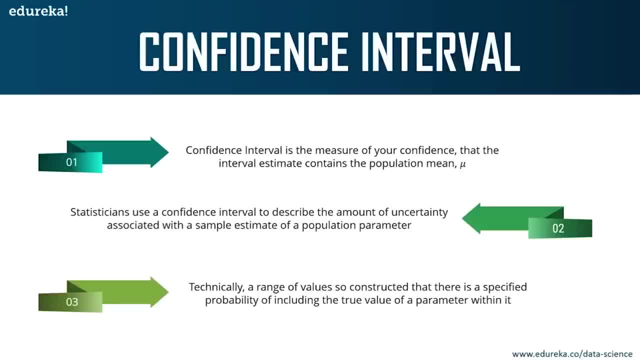 confidence level is 99% shows that you're very confident that the results are correct. Okay, I hope all of you are clear with that. All right, So your confidence interval here will be 100 and 200 and your confidence level will be 99%. right, 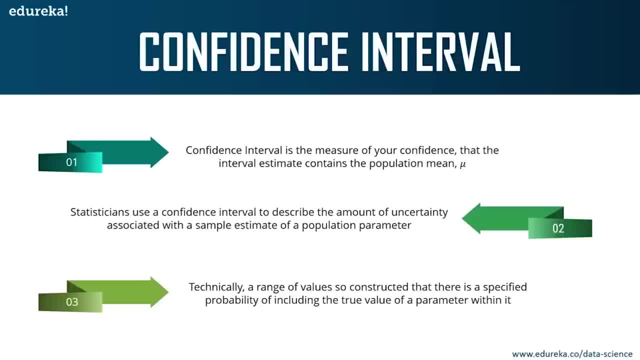 That's the difference between confidence interval and confidence level. So within your confidence interval your value is going to lie and your confidence level will show how confident you are about your estimation right? I hope that was clear. Let's look at margin of error. 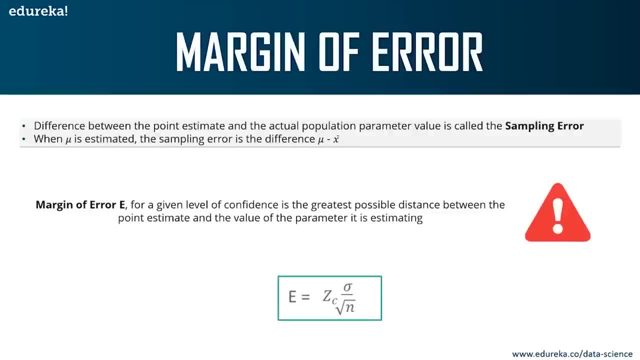 Now, margin of error for a given level of confidence is the greatest possible distance between the point estimate and the value of the parameter that it is Is estimating. you can say that it is a deviation from the actual point estimate. right now, The margin of error can be calculated using this formula. 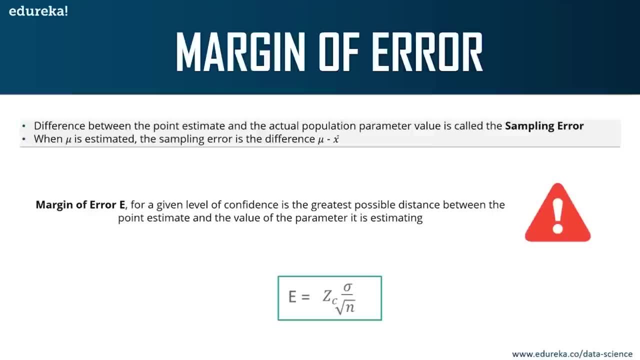 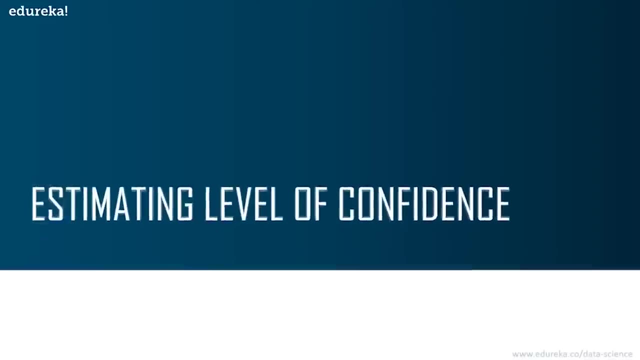 Now ZC. her denotes the critical value, or the confidence interval, and this is multiplied by standard deviation, divided by root of the sample size. All right, n is basically the sample size. Now let's understand how you can estimate the confidence intervals. So, guys, the level of confidence which is denoted by 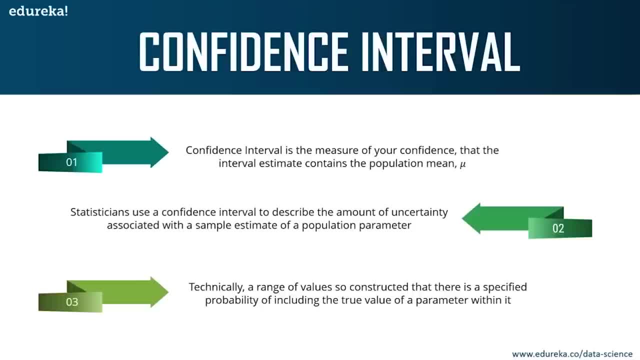 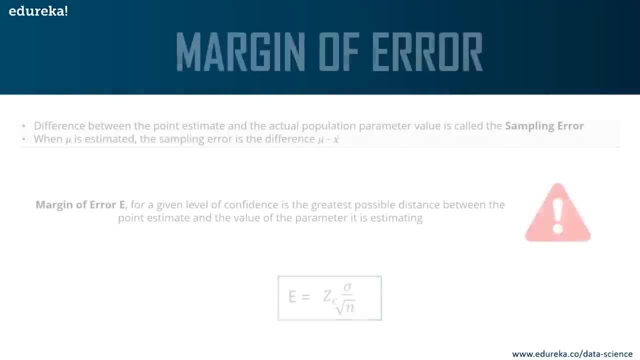 and confidence level. So within your confidence interval your value is going to lie and your confidence level will show how confident you are about your estimation right? I hope that was clear. Let's look at margin of error Now. margin of error for a given level of confidence. 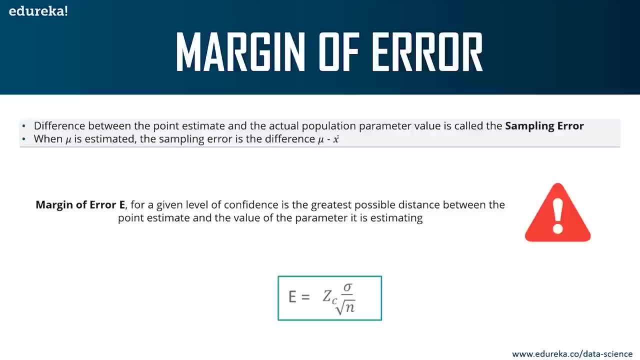 is the greatest possible distance between the point estimate and the value of the parameter that it is estimating. You can say that it is a deviation from the actual point estimate. right Now. the margin of error can be calculated using this formula Now: ZC here denotes the critical value. 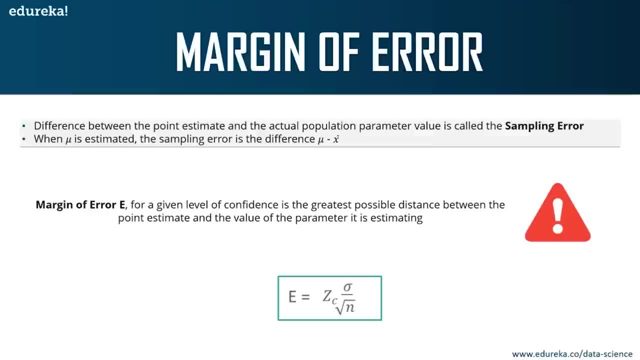 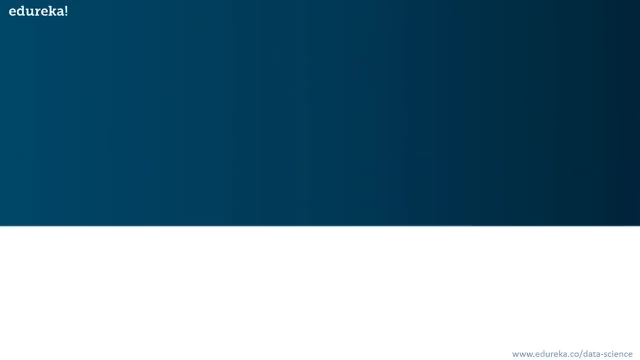 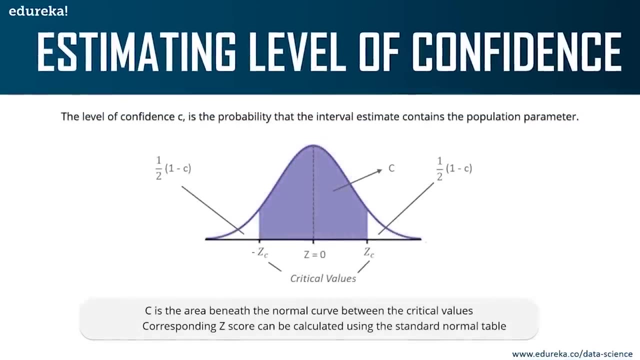 or the confidence interval, and this is multiplied by standard deviation, divided by root of the sample size. all right, N is basically the sample size. Now let's understand how you can estimate the confidence intervals. So, guys, the level of confidence which is denoted by C. 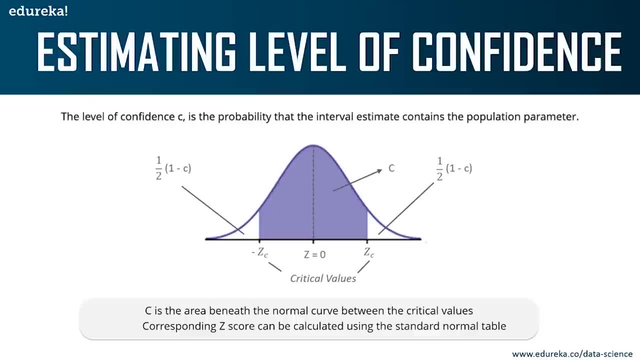 is the probability that the interval estimate contains the population parameter. Let's say that you're trying to estimate the mean, all right. So the level of confidence is the probability that the interval estimate contains the population parameter. So this interval between minus ZC and ZC. 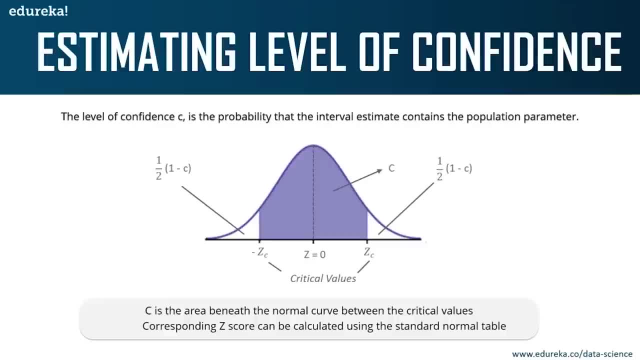 or the area beneath this curve, is nothing but the probability that the interval estimate contains the population parameter. all right. It should basically contain the value that you're predicting right Now. these are known as critical values. This is basically your lower limit. 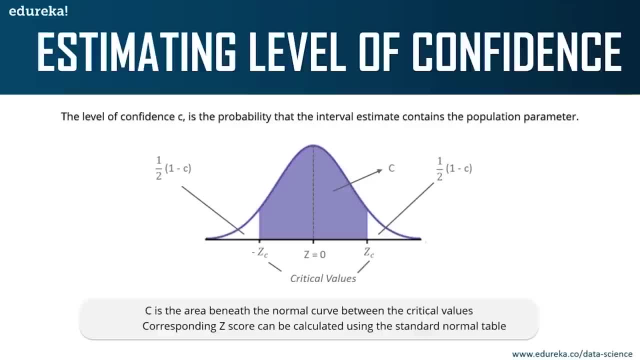 and your higher limit confidence level. Also, there's something known as the Z-score. Now, this score can be calculated by using the standard normal table. all right, If you look it up anywhere on Google, you'll find the Z-score table or the standard normal table. 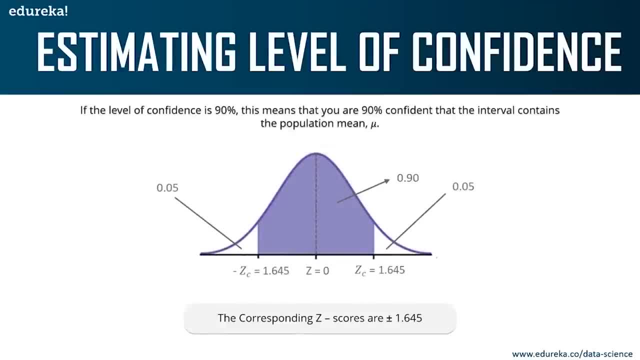 Okay, to understand how this is done, let's look at a small example. Okay, let's say that the level of confidence is 90%. This means that you are 90% confident. This means that you are 90% confident. 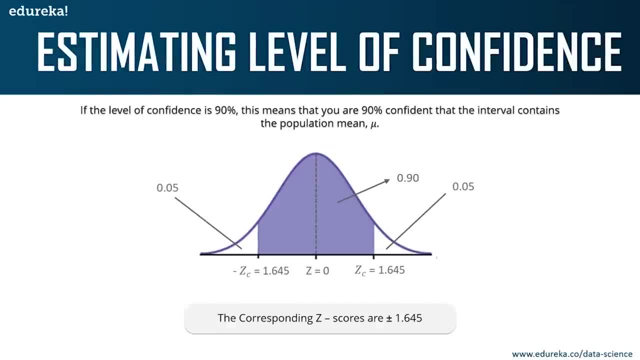 This means that you are 90% confident that the interval contains the population mean: okay, So the remaining 10%, which is out of 100%, the remaining 10% is equally distributed on these tail regions. okay, So you have 0.05 here and 0.05 over here, right? 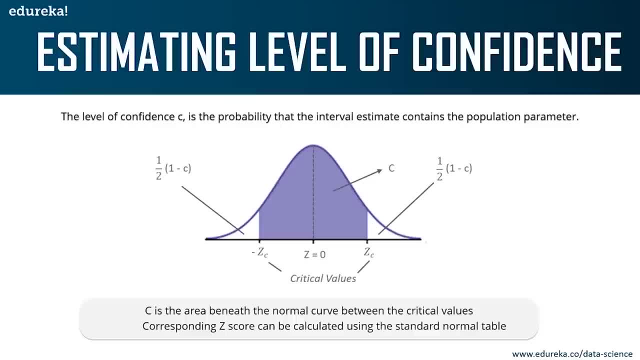 ZC is the probability that the interval estimate contains the population parameter. Let's say that you're trying to estimate the mean, all right. So the level of confidence is the probability that the interval estimate contains the population parameter. So this interval between minus ZC and ZC, or the area beneath this curve, is nothing but the probability that. 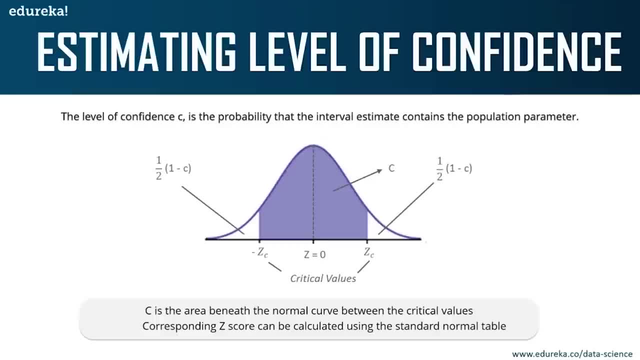 the interval estimate contains the population parameter, All right. it should basically contain the value That you are predicting right now. These are known as critical values. This is basically your lower limit and your higher limit confidence level. Also, there's something known as the Z score. 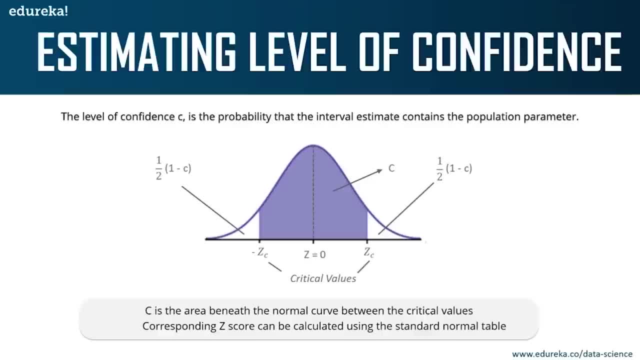 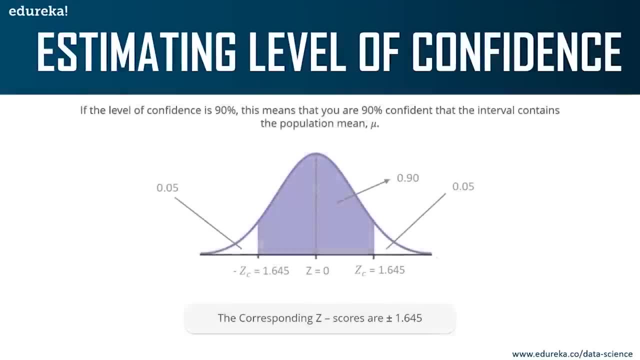 Now this code can be calculated by using the standard normal table. All right, if you look it up anywhere on Google, you'll find the Z score table or the standard normal table. get to understand how this is done, Let's look at a small example. 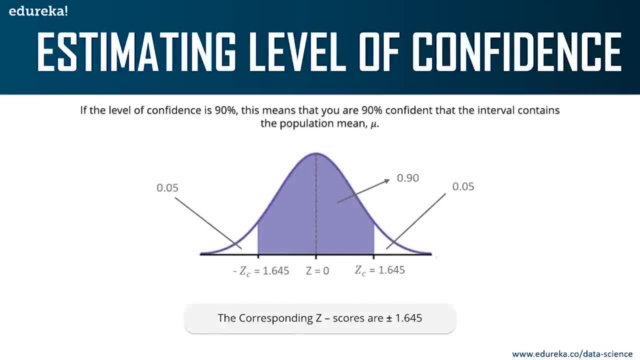 Okay, let's say that the level of confidence is 90%. This means that you are 90% confident that the interval contains the population mean. Okay, so the remaining 10%, which is out of hundred percent. The remaining 10% is equally distributed on these tail regions: 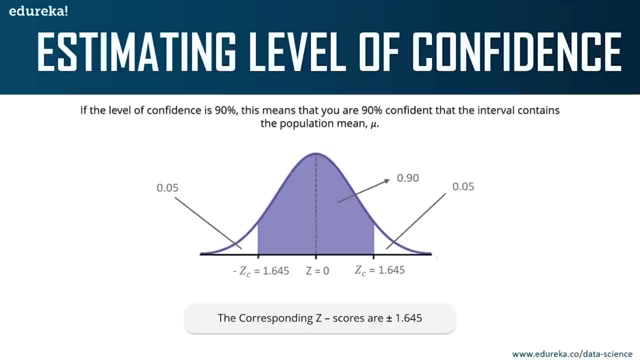 Okay, so you have 0.05 here and 0.05 over here, right? So on either side of C you'll distribute the other left over percentage. Now, these these codes are calculated from the table, as I mentioned before. All right, 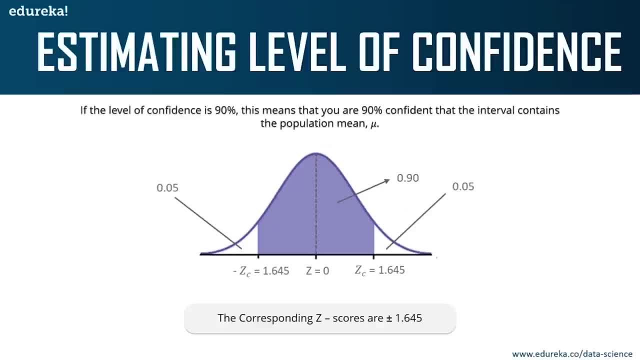 1.645 is calculated from the Standard normal table. Okay, so, guys, this is how you estimate the level of confidence. So, to sum it up, let me tell you the steps that are involved in constructing a confidence interval. First, 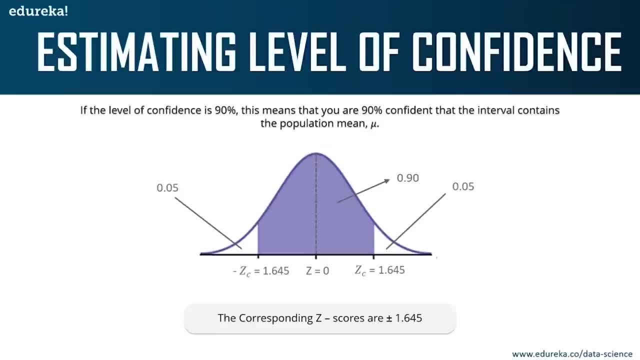 you'll start by identifying a sample statistic. Okay, this is the statistic that you will use to estimate a population parameter. This can be anything like the mean of the sample. Next, you will select a confidence level. Now, the confidence level describes the uncertainty of a sampling method. 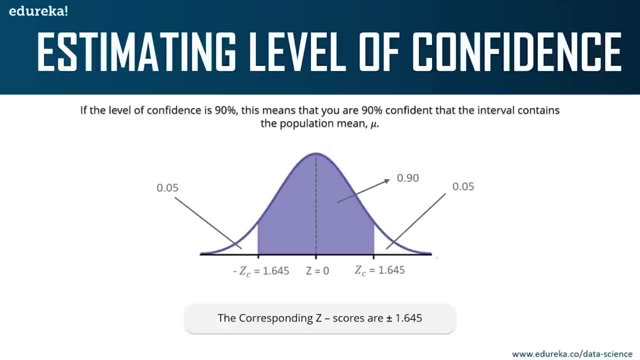 right. After that, you'll find something known as the margin of error, right? We discussed margin of error earlier, So you find this based on the equation that I explained in the previous slide. Then you'll finally specify the confidence interval. All right. 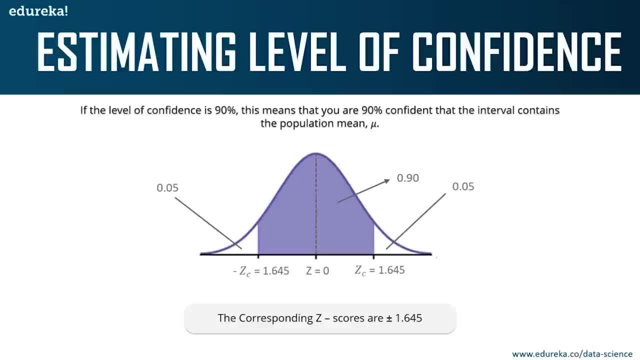 So on either side of C you'll distribute the other left over percentage. Now these Z-scores are calculated from the table, as I mentioned before. all right, 1.645 is calculated from the standard normal table. 1.645 is calculated from the standard normal table. 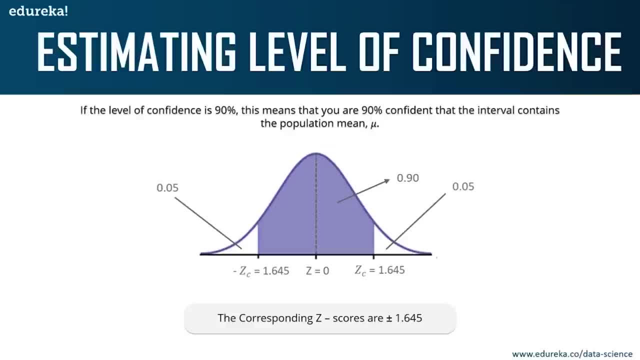 1.645 is calculated from the standard normal table. okay, So, guys, this is how you estimate the level of confidence. So, to sum it up, let me tell you the steps that are involved in constructing a confidence interval. First, you'll start by identifying a sample statistic. 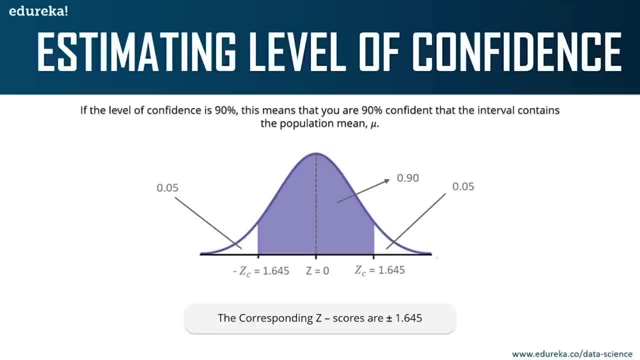 Okay, this is the statistic that you will use to estimate a population parameter. This can be anything like the mean of the sample. Next, you will select a confidence level. Now, the confidence level describes the uncertainty of a sampling method, right? 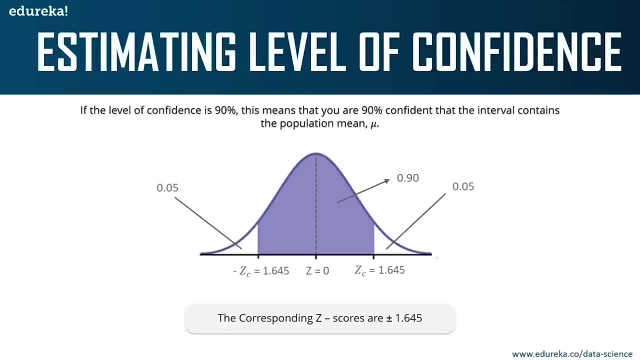 After that, you'll find something known as the margin of error. right? We discussed margin of error earlier, So you find this based on the equation that I explained in the previous slide. Then you'll finally specify the confidence interval. all right. 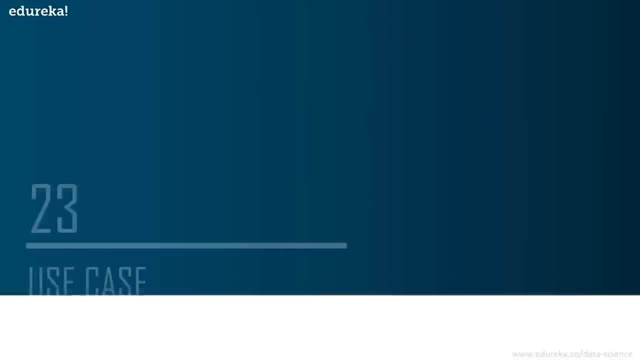 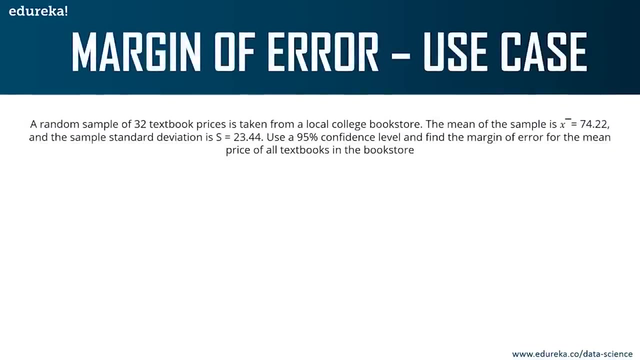 Now let's look at a problem statement to better understand this concept. A random sample of 32 textbook prizes is taken from a local college bookstore. The mean of the sample is so, so and so, and the sample standard deviation is this: 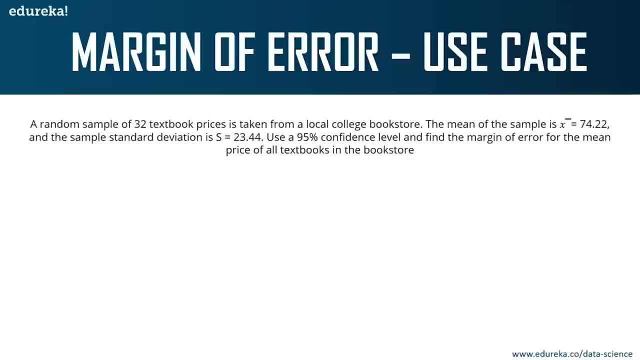 Use a 95% confident level and find the margin of error for the mean prize of all textbooks in the bookstore. okay, Now, this is a very straightforward question. If you want, you can read the question again. All you have to do is you have to just substitute. 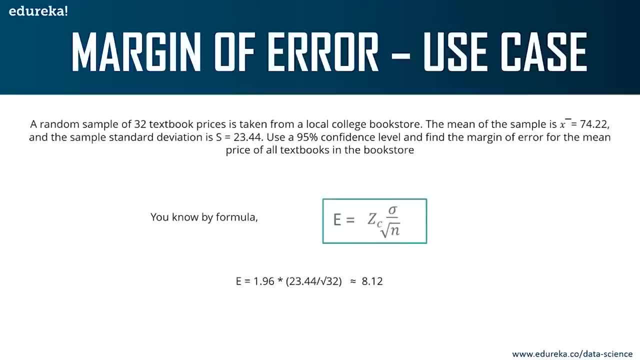 the values into the equation, all right. So, guys, we know the formula for margin of error. You take the z-score from the table. After that we have deviation which is 23.44, right, That's standard deviation, and n stands for the. 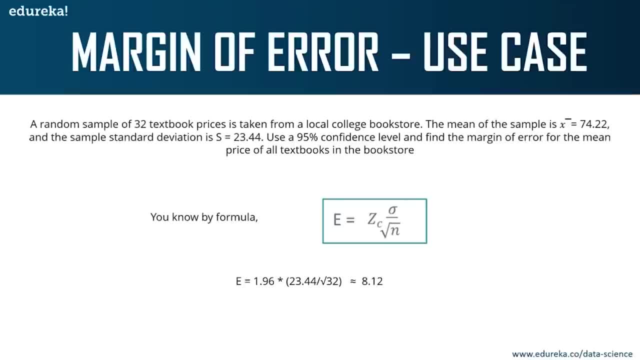 number of samples? Now the number of samples is 32, basically 32 textbooks. So approximately, your margin of error is going to be around 8.12.. This is a pretty simple question. all right, I hope all of you understood this. 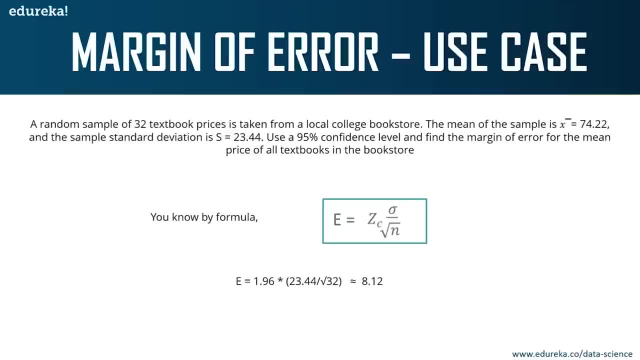 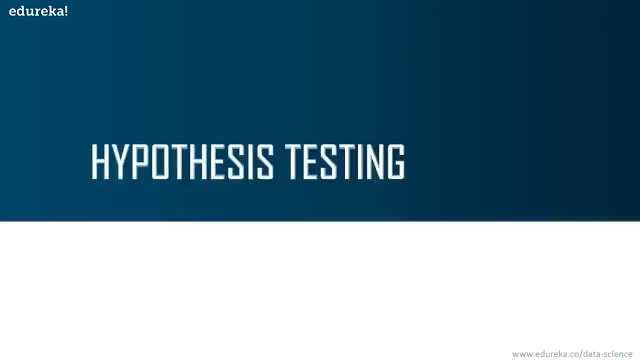 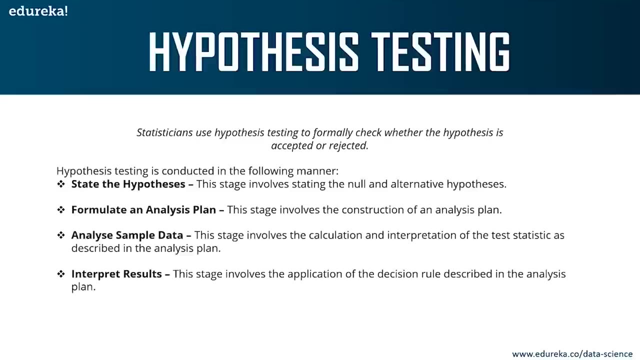 Now that you know the idea behind confidence interval, let's move ahead to one of the most important topics in statistical inference, which is hypothesis testing. right? So basically, statisticians use hypothesis testing to formally check whether the hypothesis is accepted or rejected. okay, 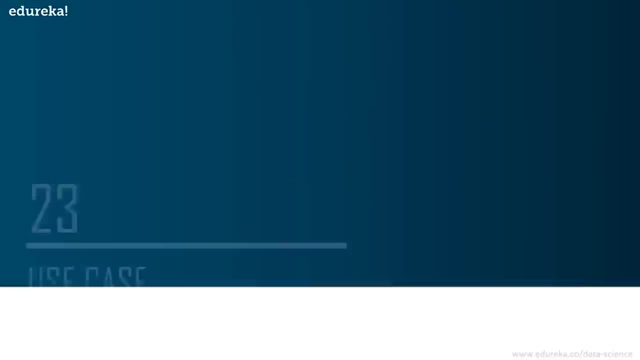 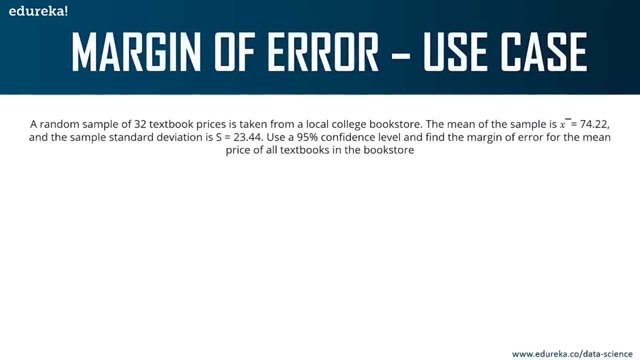 Now let's look at a problem statement to better understand this concept. A random sample of 32 textbook prices is taken from a local college bookstore. The main of the sample is so, so and so, and the sample standard deviation is this: use a 95%. 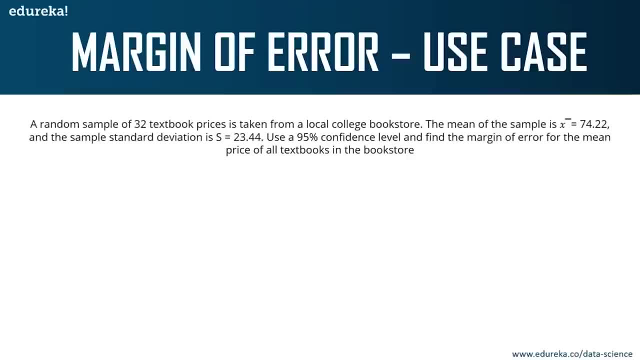 confident level and find the margin of error for the mean price of all textbooks in the bookstore. Okay, Now, this is a very straightforward question. If you want, you can read the question again. All you have to do is you have to just substitute the values into the equation. 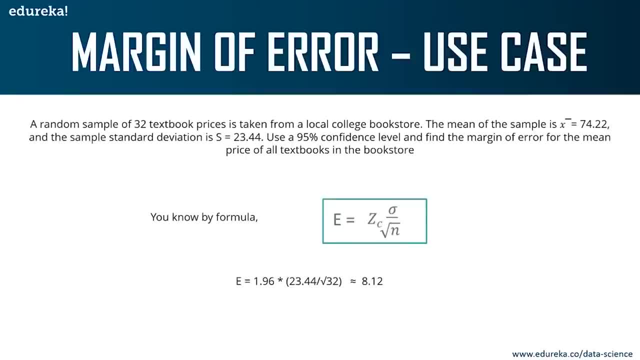 All right. So, guys, we know the formula for margin of error. You take the z-score from the table. After that we have deviation which is 23.44,. right, That's standard deviation, And n stands for the number of samples. 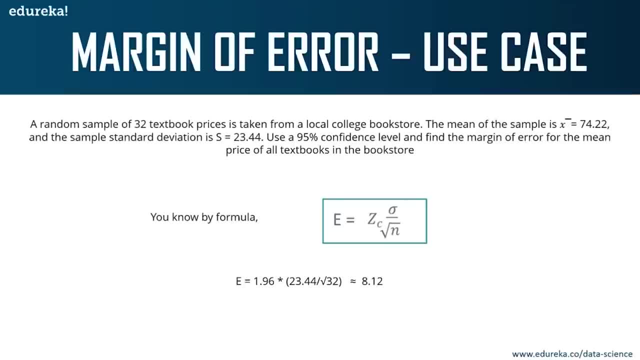 Now the number of samples is 32, basically 32 textbooks. So approximately your margin of error is going to be around 8.12.. This is a pretty simple question, All right, I hope all of you understood this, Now that you know the idea behind confidence interval. 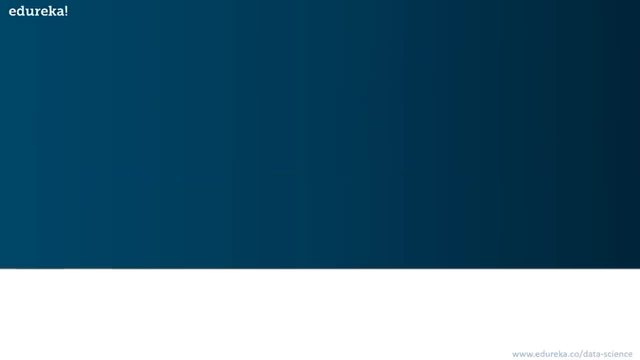 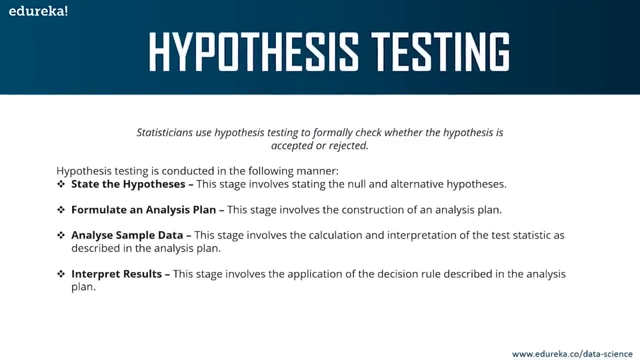 Let's move ahead to one of the most important topics in statistical inference, which is hypothesis testing. right? So basically, statisticians use hypotheses. This is testing to formally check whether the hypothesis is accepted or rejected. Okay, hypothesis testing is an inferential statistical technique used to determine whether there is enough evidence in a data sample to infer that a certain condition holds true for an entire population. 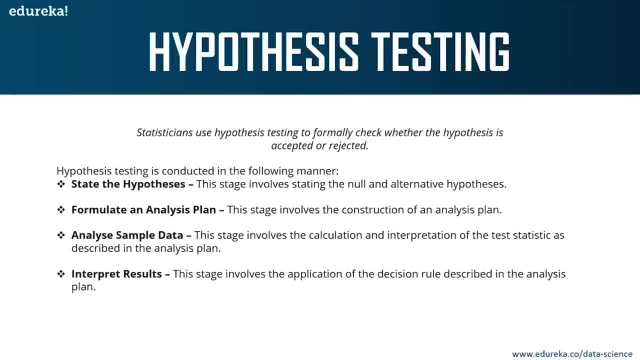 So, to understand the characteristics of a general population, we take a random sample and we analyze the properties of the sample right, We test whether or not the identified Conclusion represents the population accurately And finally we interpret their results. Now, whether or not to accept the hypothesis depends upon the percentage value that we get from the hypothesis. 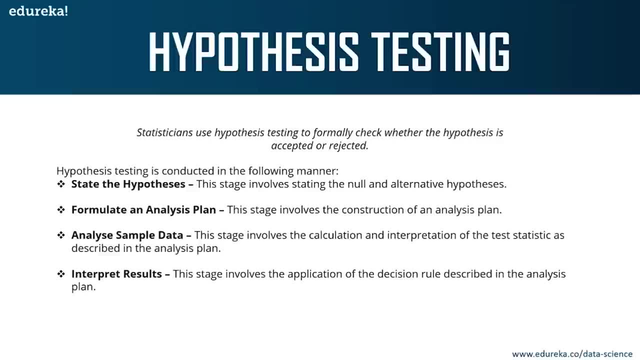 Okay, so to better understand this, let's look at a small example. Before that, there are a few steps that are followed in hypothesis testing. You begin by stating the null and the alternative hypothesis- All right, I'll tell you what exactly these terms are- and then you formulate an analysis plan. 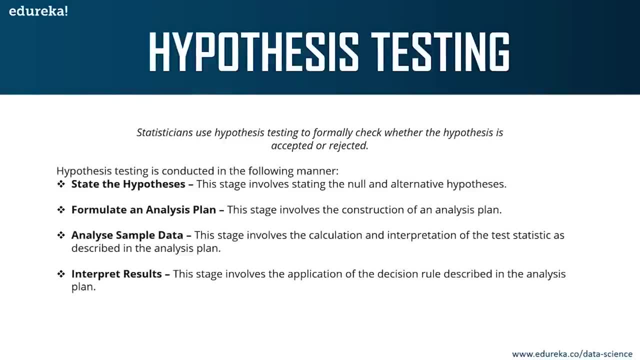 Hypothesis testing is an inferential statistical technique used to determine whether there is enough evidence in a data sample to infer that a certain condition holds true for an entire population. So to understand the characteristics of a general population, we take a random sample. 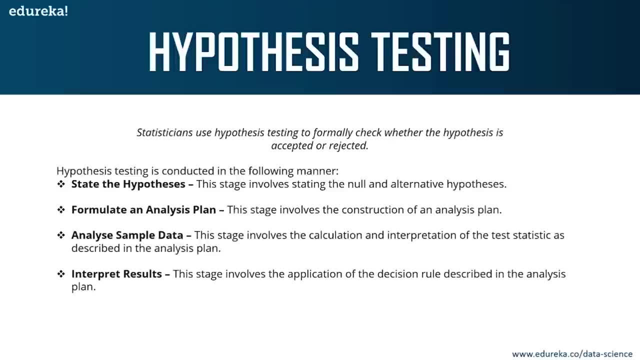 and we analyze the properties of the sample right, We test whether or not the identified conclusion represents the population accurately and finally, we interpret their results. Now, whether or not to accept the hypothesis depends upon the percentage value that we get from the hypothesis. 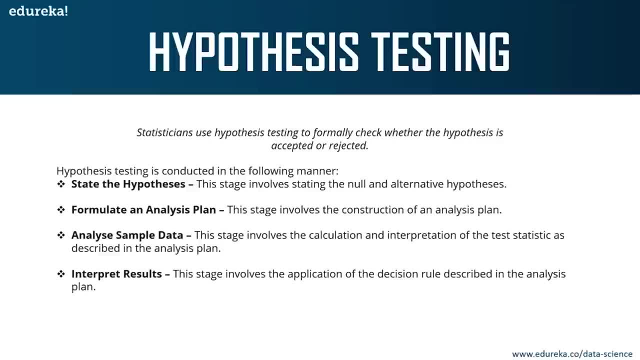 Okay, so to better understand this, let's look at a small example. Before that, there are a few steps that are followed in hypothesis testing. You begin by stating the null and the alternative hypothesis. all right, I'll tell you what exactly these terms are. 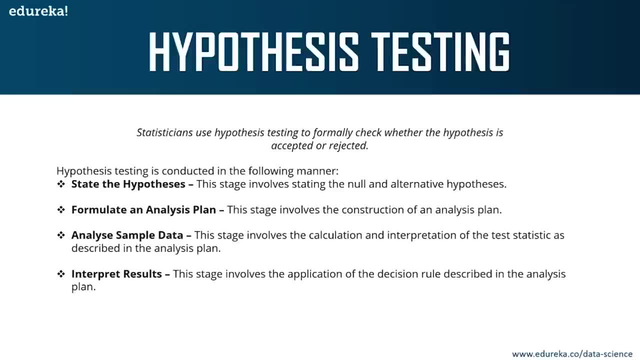 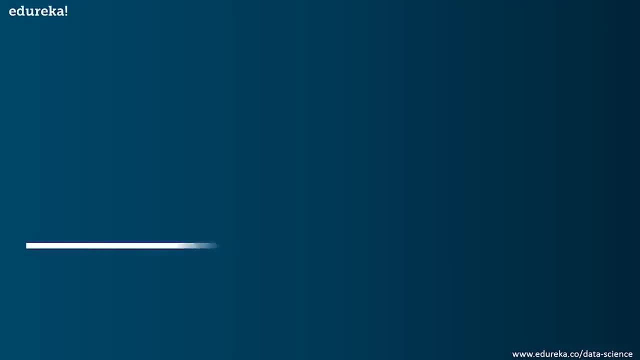 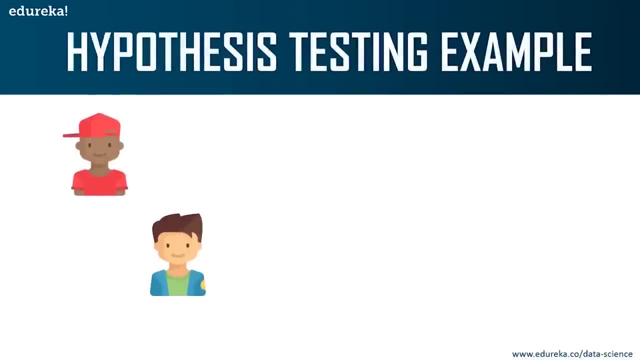 and then you formulate an analysis plan, all right. After that you analyze the sample data and finally, you can interpret the results right Now to understand the entire hypothesis testing, we'll look at a good example. okay, Now consider four boys: Nick, John, Bob and Harry. 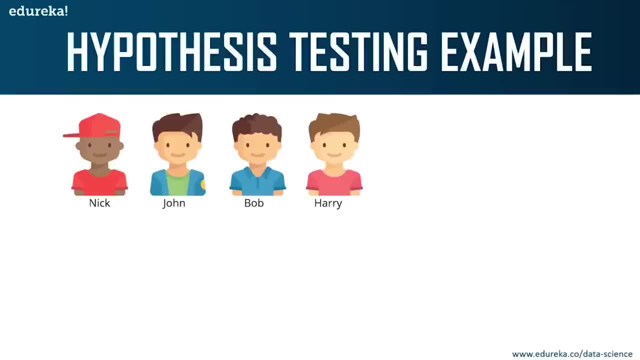 These boys were caught bunking a class and they were asked to stay back at school and clean their classroom as a punishment right. So what John did is he decided that four of them would take turns to clean their classrooms. He came up with a plan. 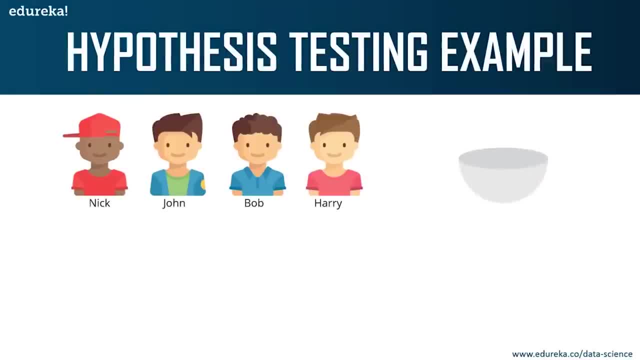 of writing each of their names on chits and putting them in a bowl. Now, every day they had to pick up a name from the bowl and that person had to clean the class, right? That sounds pretty fair enough. Now it has been three days. 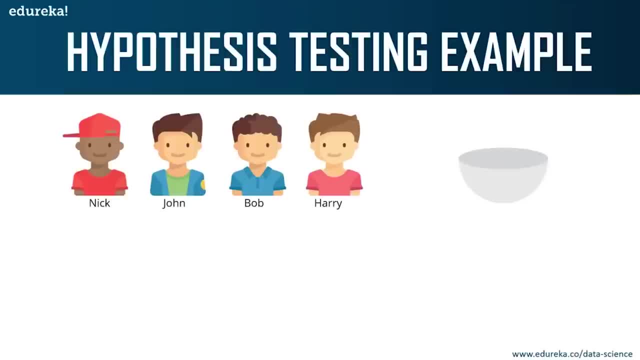 and everybody's name has come up except John's. Assuming that this event is completely random and free of bias, what is the probability of John not cheating, right? What is the probability that he's not actually cheating? This can be solved by using a name: Chi-Gen, okay. This can be solved by using a name: Chi-Gen right. Why John one years ago wasn't he cheating? What is the probability that he was not cheating? Why John one years ago wasn't he cheating? Why John one years ago wasn't he cheating? There was not going to take the class topic, which was not cheating. 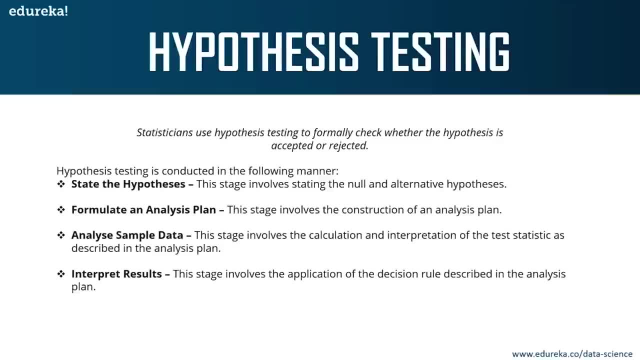 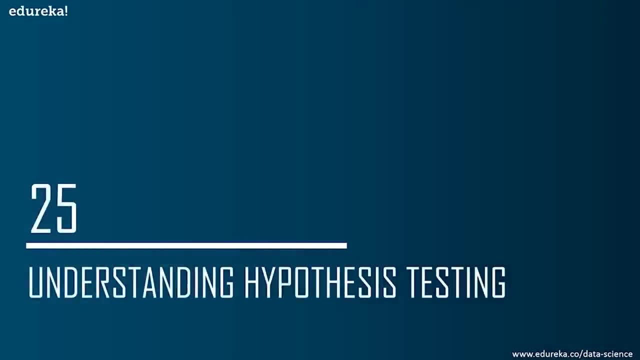 All right. after that, you analyze the sample data and finally, you can interpret the results right Now to understand the entire hypothesis testing, we look at a good example. Okay, now consider four boys: Nick, John, Bob and Harry. 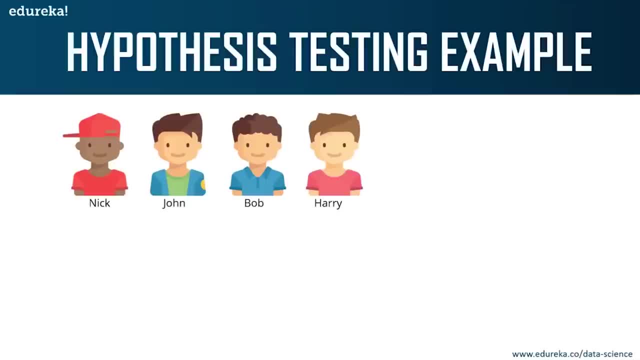 These boys were caught bunking a class and they were asked to stay back at school and clean their classroom as a punishment Right. So what John did is he decided that four of them would take turns to clean their classrooms. He came up with a plan of writing each of their names on chits and putting them in a bowl. 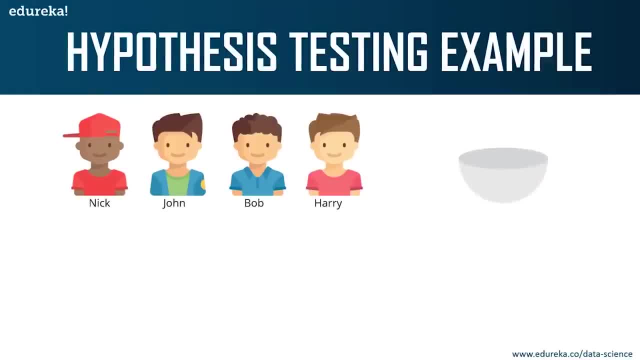 Now, every day they had to pick up a name from the bowl and that person had to clean the class, right? That sounds pretty fair enough. Now it has been three days and everybody's name has come up except John's, Assuming that this event is completely random and free of bias. 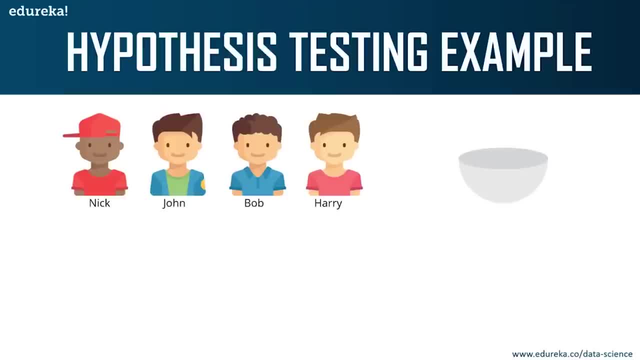 What is the probability of John not cheating, Right? What is the probability that he's not actually cheating? This can be solved by using hypothesis testing. Okay, so we'll begin by calculating the probability of John not being picked for a day, Right. 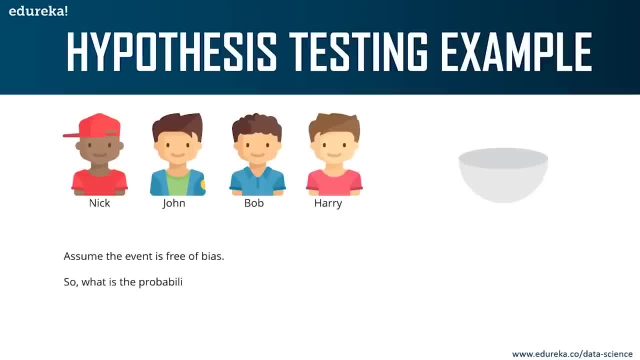 So we're going to assume that the event is free of bias. So we need to find out the probability of John not cheating Right First. we'll find the probability that John is not picked for a day Right, We get three out of four. 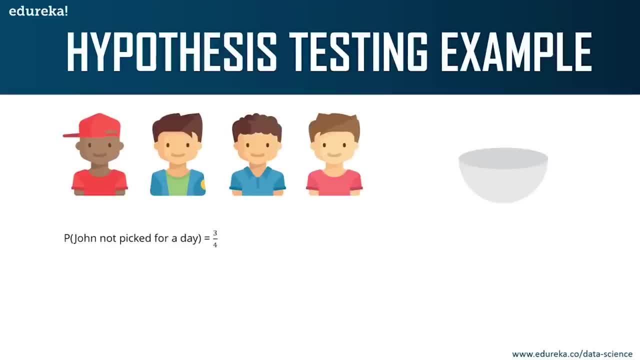 which is basically 75% of 75%, is fairly high. So if John is not picked for three days in a row, the probability will drop down to approximately 42%. Okay, so three days in a row, meaning that is, the probability drops down to 42%. 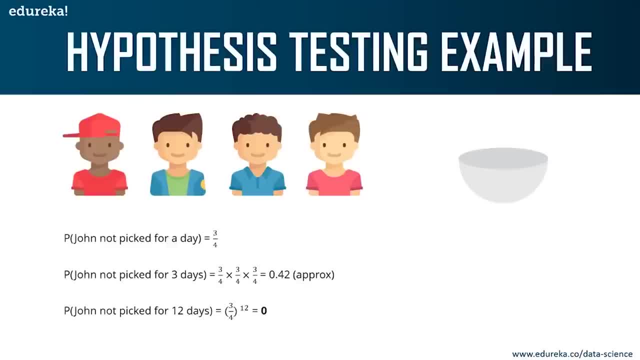 Now let's consider a situation where John is not picked for 12 days in a row. The probability drops down to 3.2%. Okay, that's, the probability of John cheating becomes fairly high, Right? So, in order for statisticians to come to a conclusion, 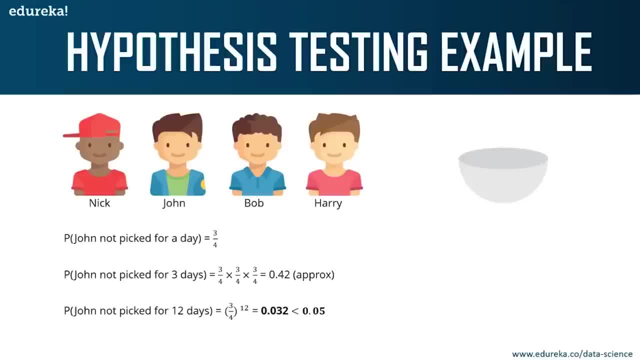 they define what is known as the threshold value Right. Considering the above situation, if the threshold value is set to 5%, it would indicate that if the probability lies below 5%, then John is cheating his way out of detention, But if the probability is about threshold value, 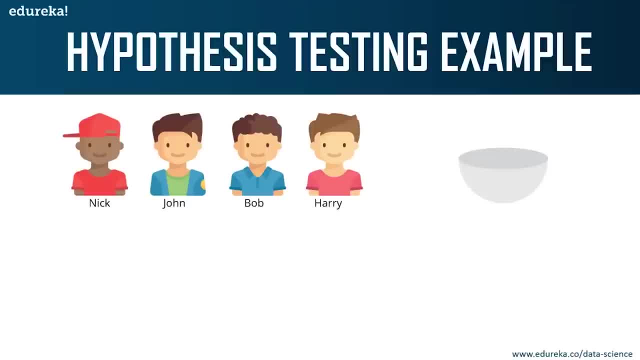 hypothesis testing. okay, so we'll begin by calculating the probability of john not being picked for a day, right? so we're going to assume that the event is free of bias. so we need to find out the probability of john not cheating right first. we'll find the probability that john is not. 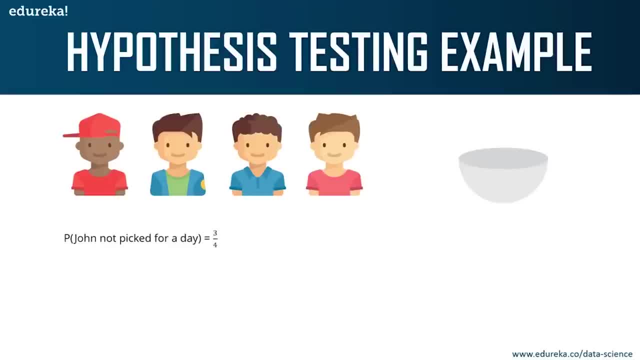 picked for a day. right, we get three out of four, which is basically 75 percent. now, 75 percent is fairly high, so if john is not picked for three days in a row, the probability will drop down to approximately 42 percent. okay, so three days in a row, meaning that is, the probability drops down to. 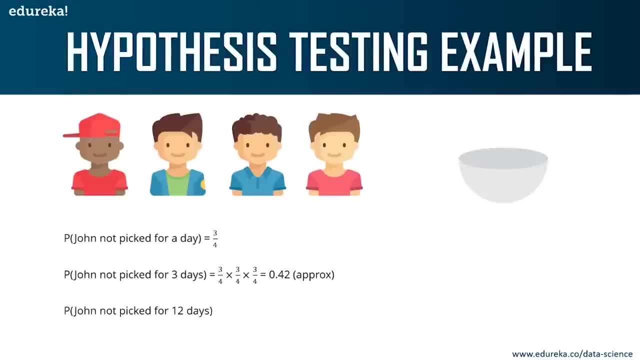 42 percent. now let's consider a situation where john is not picked for 12 days in a row. the probability drops down to 3.2 percent. okay, that's, the probability of john cheating becomes fairly high, right? so in order for step statisticians to come to a conclusion, they define what is known as the threshold value. 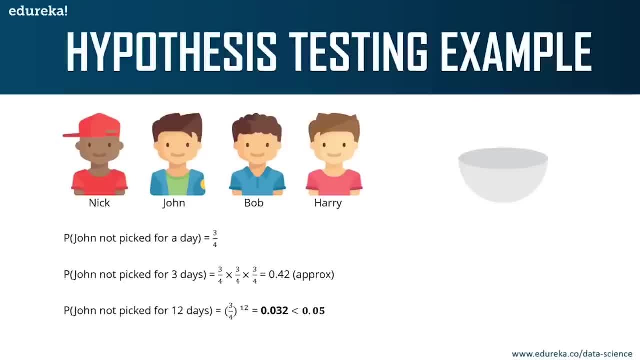 right, considering the above situation. if the threshold value is set to five percent, it would indicate that if the probability lies below five percent, then john is cheating his way out of detention, but if the probability is above threshold value, then john is just lucky and his name isn't. 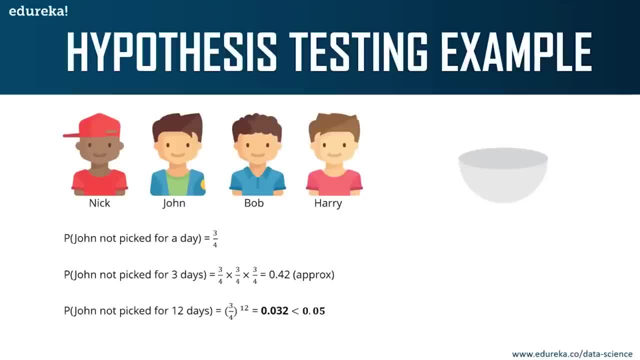 getting picked. so the probability and hypothesis testing give rise to two important components of hypothesis testing, which is not null hypothesis and alternate hypothesis. null hypothesis is basically approving the assumption. alternate hypothesis is when your result disapproves the assumption right. therefore, in our example, if the probability of an event occurring is less than five percent, which it is, then the event is biased. 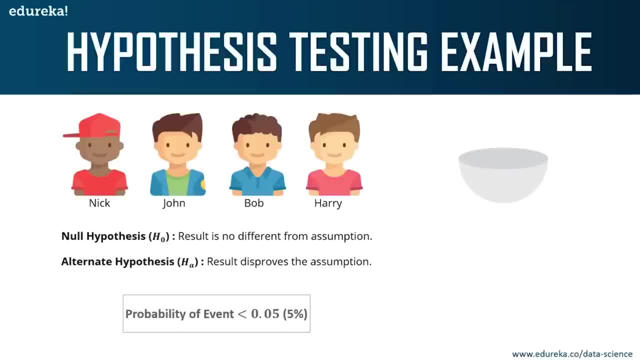 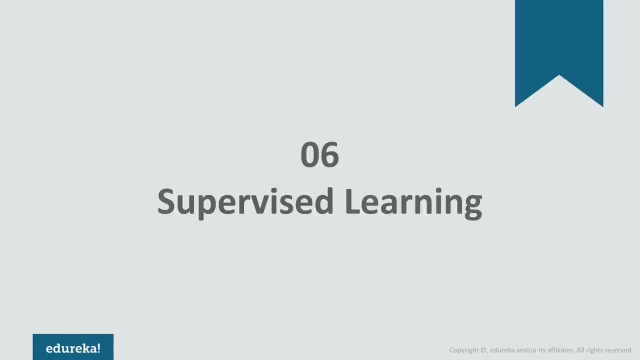 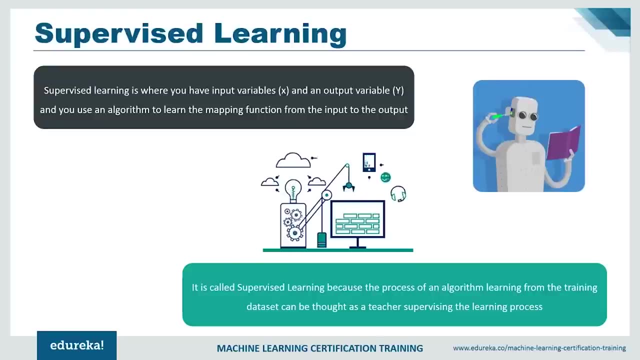 hence it proves the alternate hypothesis. so, guys, with this we come to the end of this session. let's go les, go ahead and sand what exactly is supervised learning. so supervised learning is where you have the input variable x and the output radio, while kork of the map pick function from the 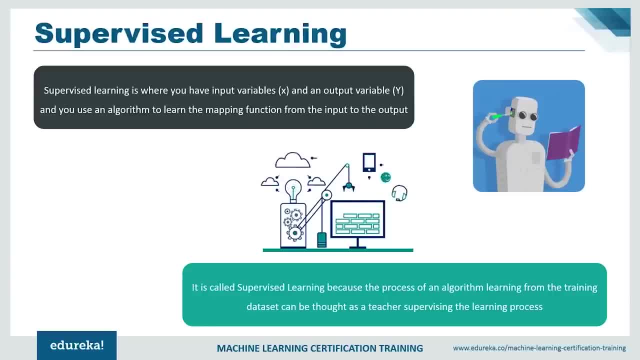 input to the out, as i mentioned earlier with the example of face detection. so it is called supervised learning, because the process of an algorithm learning from the training data set can be thought of as. So, if we have a look at the supervised learning steps, or what we would rather say, the workflow, 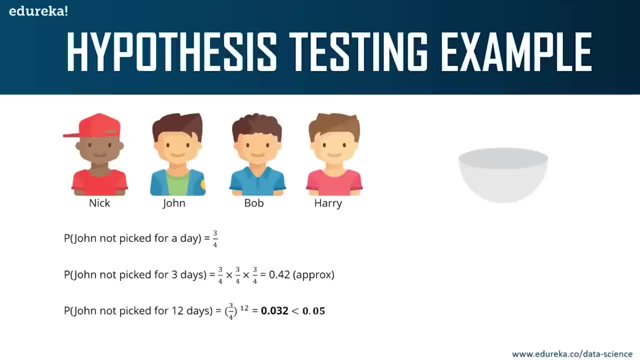 then John is just lucky and his name isn't getting picked. So the probability and hypothesis testing give rise to two important components of hypothesis testing, which is null hypothesis and alternate hypothesis. Null hypothesis is basically approving the assumption. Alternate hypothesis is when your result disapproves the assumption. 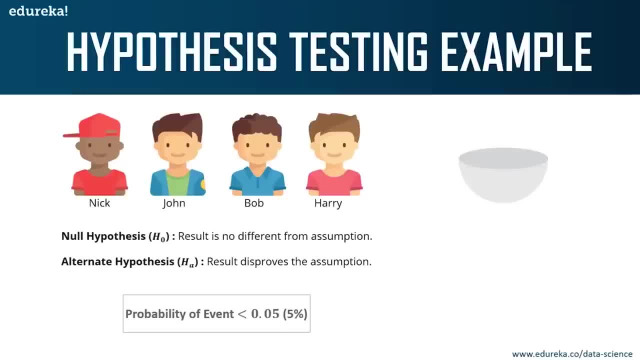 Right. Therefore, in our example, if the probability of an event occurring is less than 5%- which it is- then the event is biased, Hence it proves the alternate hypothesis. So, guys, with this we come to the end of this session. 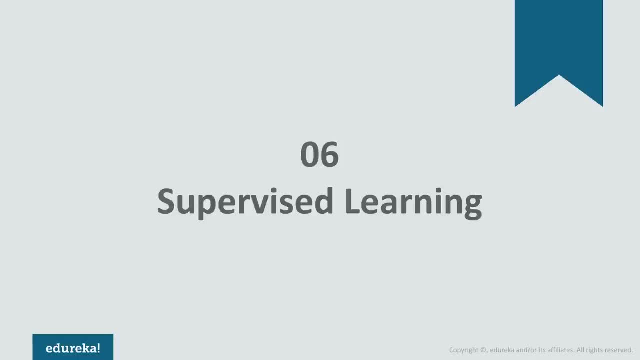 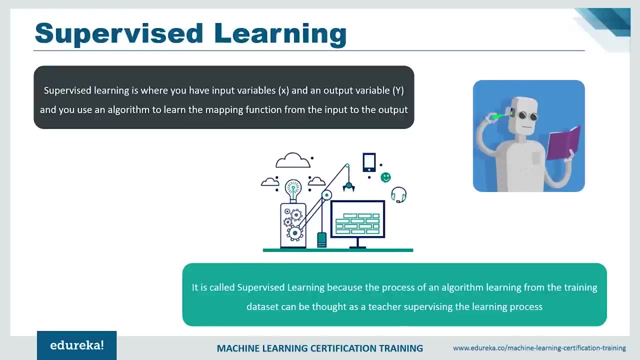 Let's go ahead and understand what exactly is Supervised learning. So supervised learning is where you have the input variable X and the output variable Y and you use an algorithm to learn the MAPIC function from the input to the output, As I mentioned earlier with the example of face detection. 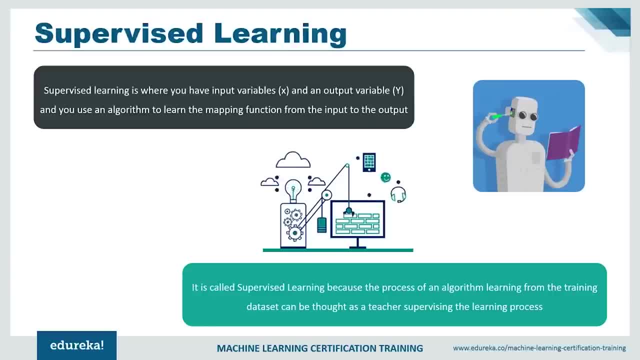 So it is called supervised learning, because the process of an algorithm learning from the training data set can be thought of as a teacher supervising the learning process. So if we have a look at the supervised learning steps, or what we'd rather say the workflow, 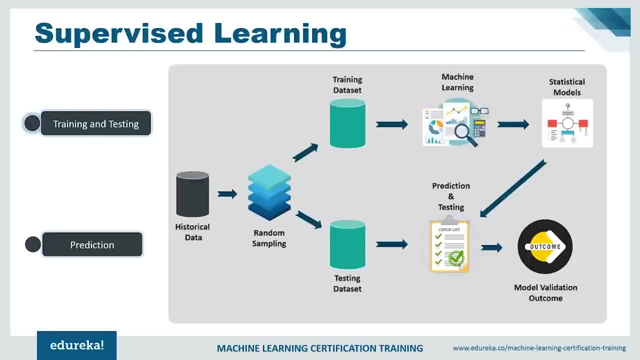 So the model is used as you can see. here We have the historic data, Then we again we have the random sampling with split the data into training data set and the testing data set. using the training data set, We, with the help of machine learning, 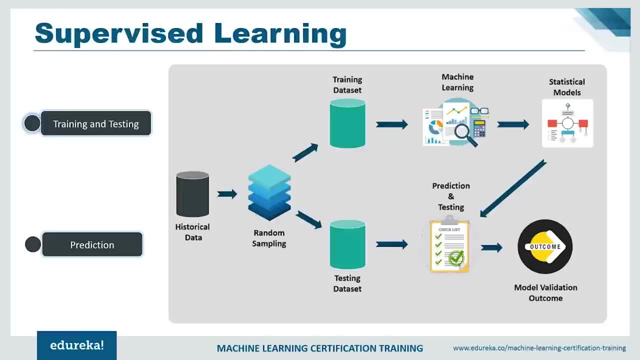 which is supervised machine learning, we create statistical model And then, after we have a model which is being generated with the help of the training data set, what we do is use the testing data set for prediction and testing. What we do is get the output and finally we have the model validation. 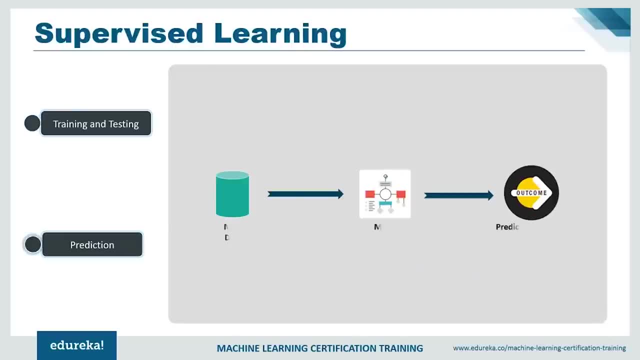 outcome. that was the training and testing. So if we have a look at the prediction part of any particular supervised learning algorithm, so the model is used for operating. outcome of a new data set. So whenever performance of the model degraded, the model is retrained or 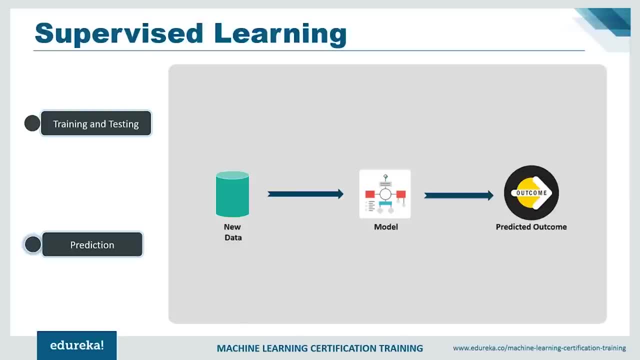 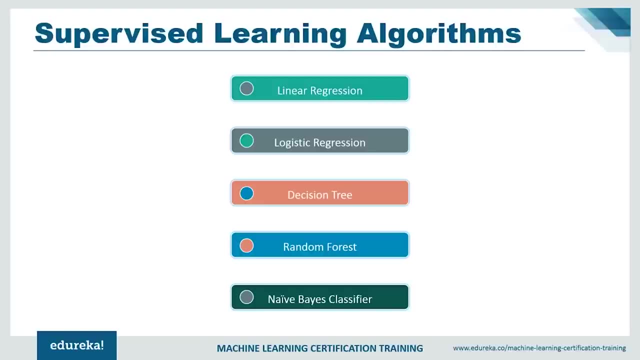 if there are any performance issues, the model is retrained with the help of the new data. Now, when we talk about supervised learning, there are not just one, but quite a few algorithms here. So we have linear regression, logistic regression, decision tree. 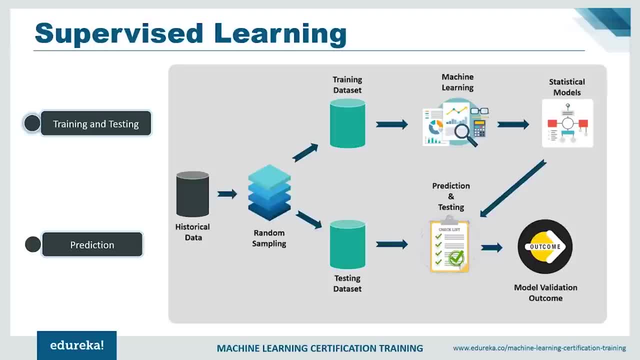 So the model is used as you can see, here we have the historic data, then we again we have the random sampling. we split the data into training data set and the testing data set. Using the training data set, we, with the help of machine learning, which is supervised machine learning, we create statistical model. 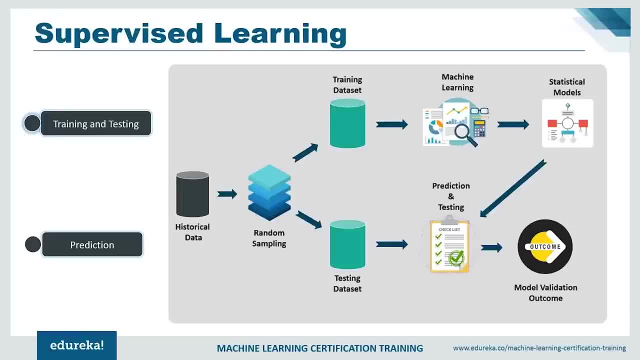 And then, after we have a model which is being generated with the help of the training data set, what we do is use the testing data set for prediction and testing. What we do is get the output and finally, we have the model validation outcome. That was the training and testing. 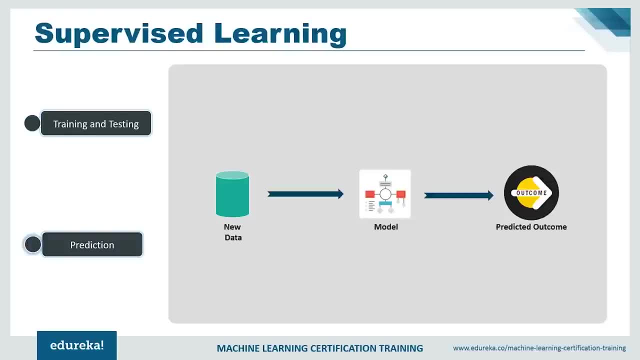 So if we have a look at the prediction part of any particular supervised learning algorithm, so the model is used for predicting outcome of a new data set. So whenever performance of the model degraded, the model is retrained. Or if there are any performance issues, the model is retrained with the help of the new data. 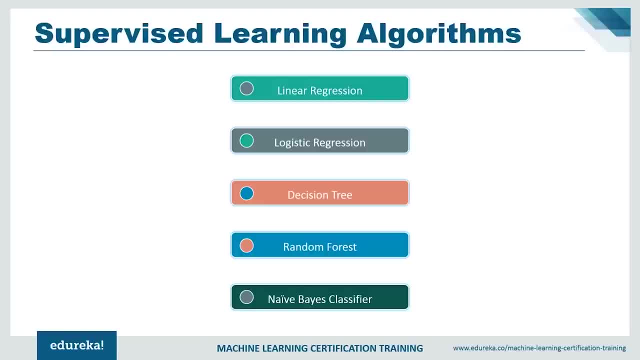 Now, when we talk about supervised learning, there are not just one but quite a few algorithms here. So we have linear regression, logistic regression decision tree, we have random forest, we have nape bias classifiers. So linear regression is used to estimate real values, for example, the cost of houses, the number of calls, the total sales, based on the continuous variables. 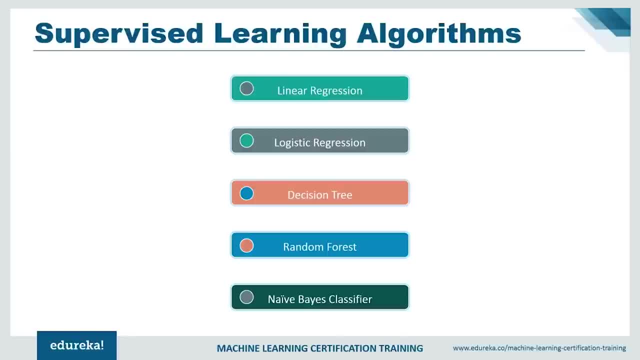 So that is what Now, when we talk about logistic regression, it is used to estimate discrete values, for example, which are binary values like 0 and 1, yes or no, true and false, based on the given set of independent variables. So, for example, when we are talking about something like the chances of winning, or if we talk about winning, which can be the true or false, will it rain today? it can be the yes or no. 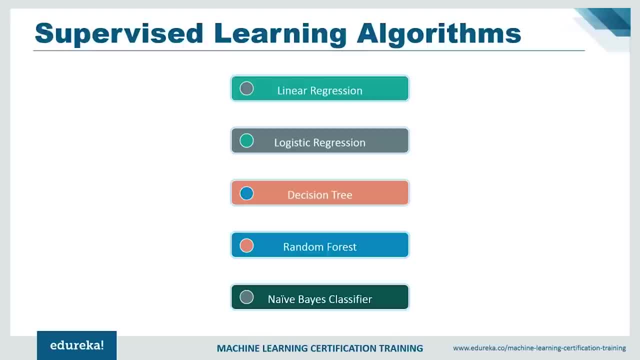 So it cannot be like when the output of a particular algorithm or the particular question Is either yes or no or a binary, then only we use a logistic regression Now. next we have decision trees, So these are used for classification problems. It works for both categorical and continuous dependent variables. 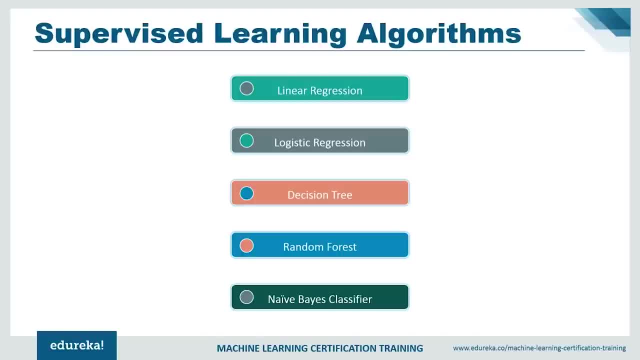 And if we talk about random forest, So random forest is an ensemble of a decision tree. It gives better prediction and accuracy than decision tree, So that is another type of supervised learning algorithm. And finally, we have the nape bias classifier, So it is a classification. 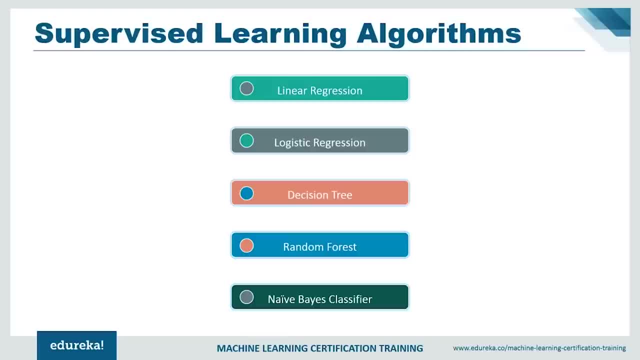 We have random Forest, We have nape bias classifiers, So linear regression is used to estimate real values, For example, the cost of houses, the number of calls, the total sales, based on the continuous variable. So that is what we need. 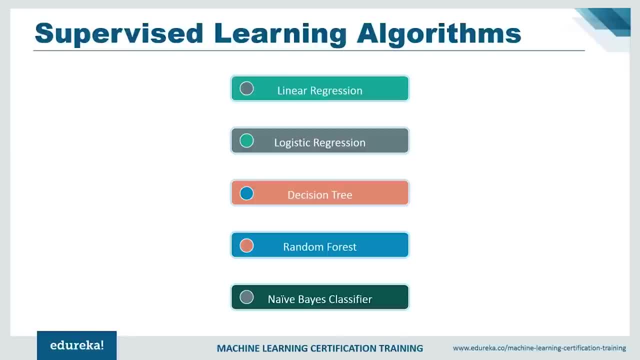 Regression is now when we talk about logistic regression. it is used to estimate discrete values, For example, which are binary values like zero and one Yes And no, true and false, based on the given set of independent variables. So, for example, when you are talking about something like the chances of winning, or if you 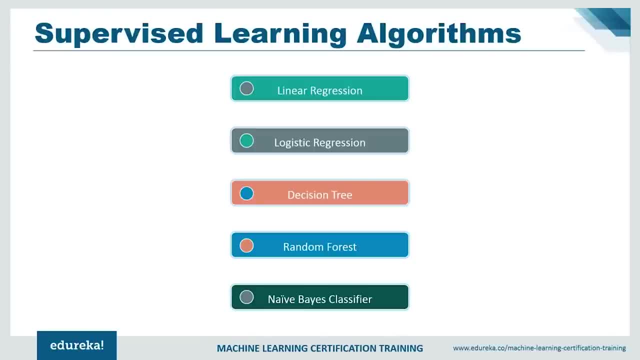 talk about winning, which can be the true or false, if will it rain today, which it can be the yes or no. So it cannot be like when the output of a particular algorithm or the particular question is either yes, no or a binary. 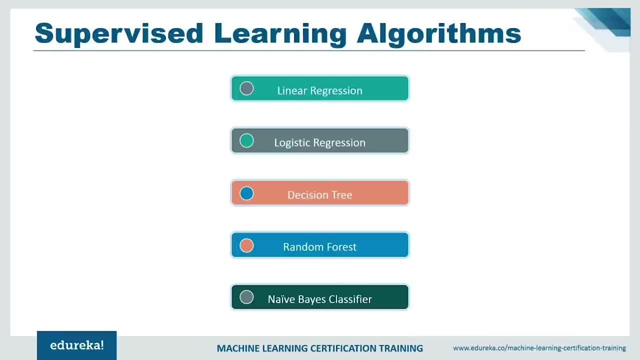 then only we use a logistic regression Now. next we have decision trees, So these are used for classification problems. It works for both categorical and continuous dependent variables, And if we talk about random forest, so a random forest is an ensemble of a decision tree. 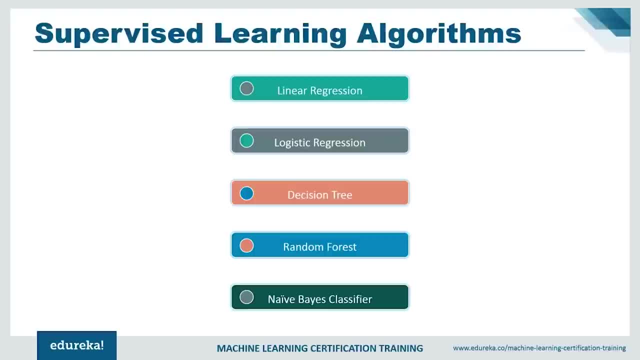 It gives better prediction and accuracy than decision tree, So that is another type of supervised learning algorithm. And finally, we have the NaPyS classifier. So it was a classification technique based on the Bayes theorem with an assumption of independence between predictors. 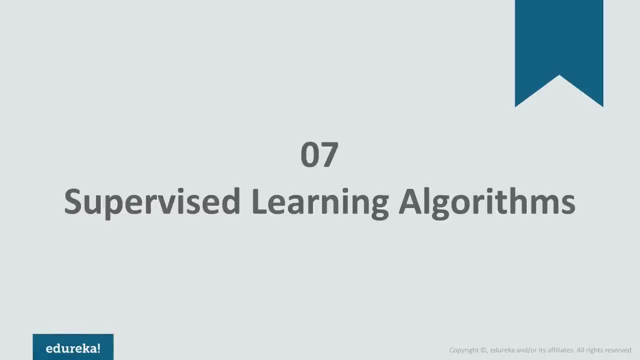 A linear regression is one of the easiest algorithm in machine learning. It is a statistical model that attempts to show the relationship between two variables with a linear equation. But before we drill down to linear regression algorithm in depth, I'll give you a quick overview of today's agenda. 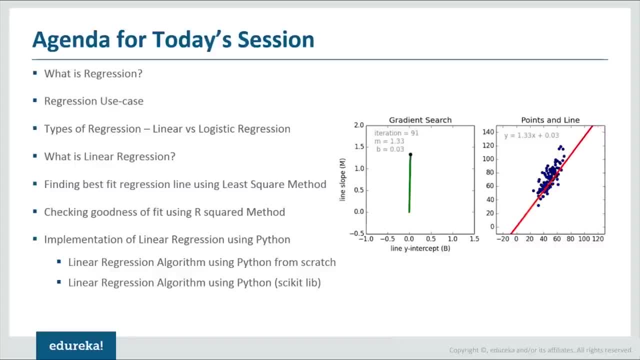 So we'll start a session with a quick overview of what is regression, as linear regression is one of a type of regression algorithm. Once we learn about regression, its use case, the various types of it, Next we'll learn about the algorithm from scratch. 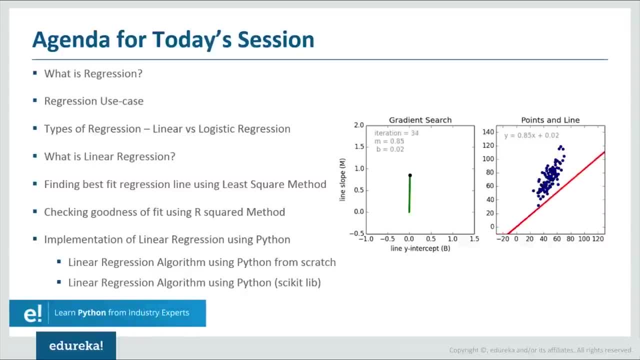 where I'll teach you its mathematical implementation first. Then we'll drill down to the coding part and implement linear regression using Python. In today's session we'll deal with linear regression algorithm using least square method. Check its goodness of fit, or how close the data is to the fitted regression line, using the R square method. 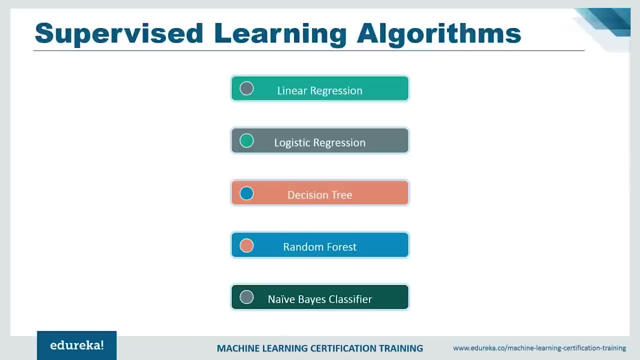 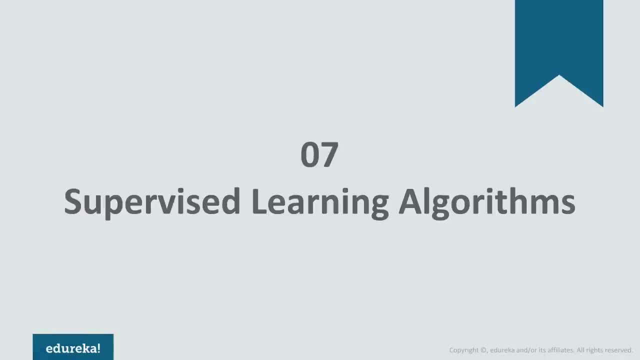 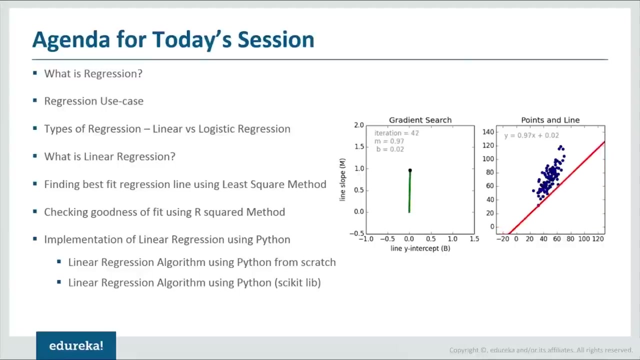 Technique based on the Bayes theorem with an assumption of independence between predictors. A linear regression is one of the easiest algorithm in machine learning. It is a statistical model that attempts to show the relationship between two variables with a linear equation. But before we drill down to linear regression algorithm in depth, I'll give you a quick overview of today's agenda. 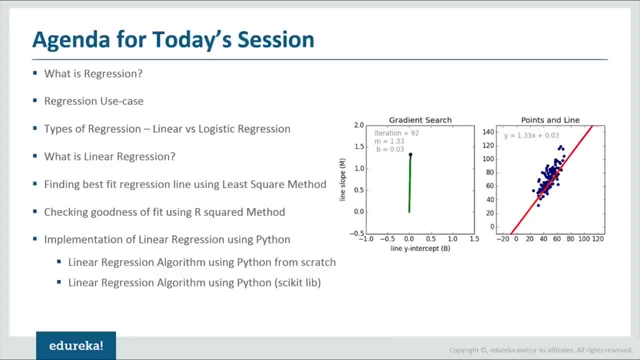 So we'll start a session with a quick overview of what is regression, As linear regression is one of a type of regression algorithm. Once we learn about regression, its use case, the various types of it, Next we'll learn about the algorithm from scratch, where I'll teach you its mathematical implementation first, 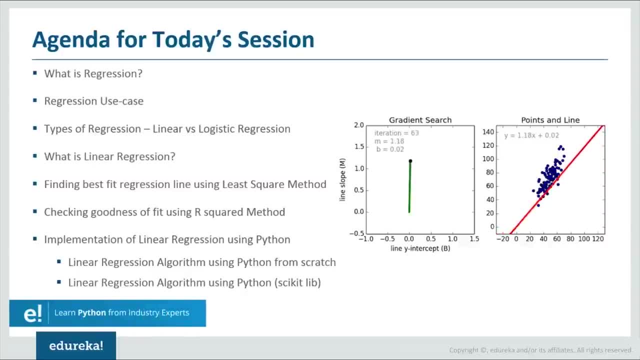 Then we'll drill down to the coding part and implement linear regression using Python. In today's session We'll deal with linear regression algorithm using least square method. check its goodness of fit or how close the data is to the fitted regression line using the r-square method. 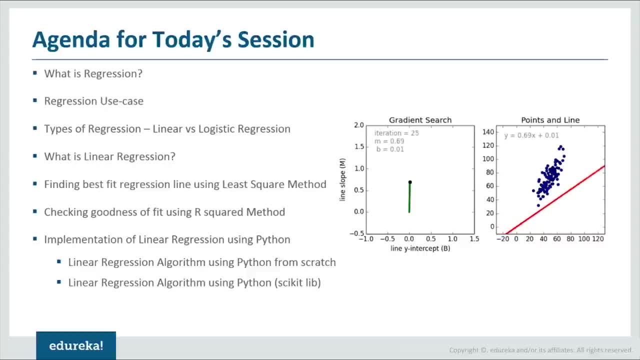 And then, Finally, what we'll do will optimize it using the gradient descent method. in the last part, on the coding session, I'll teach you to implement linear regression using Python, and the coding session would be divided into two parts. The first part would consist of linear regression using Python from scratch, where you will use the mathematical algorithm that you have learned in the session. 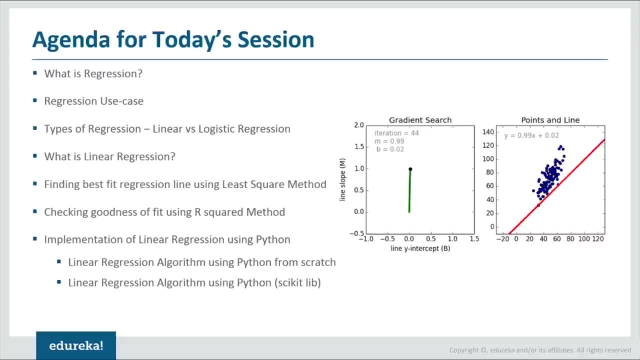 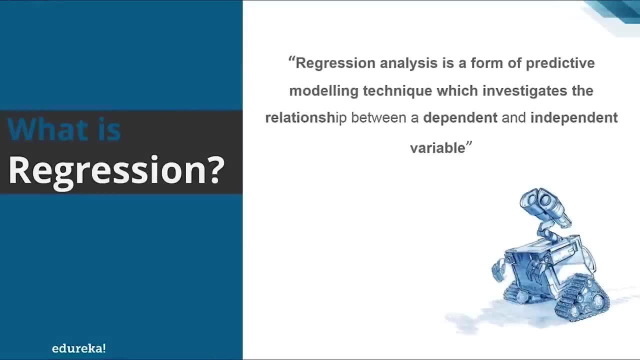 and in the next part of the coding session, will be using scikit-learn for Derek implementation of linear regression. So let's begin our session with what is regression? Well, regression analysis is a form of predictive modeling technique which investigates the relationship between a dependent and independent variable. a regression analysis involves graphing a line. 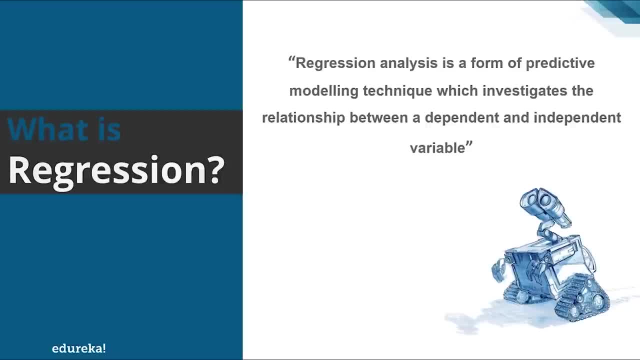 over a set of data points that most closely fits the overall shape of the data. a regression shows the changes in a dependent variable on the y-axis to the changes in the explanatory variable on the x-axis. Fine, Now you'd ask what are the uses of regression? 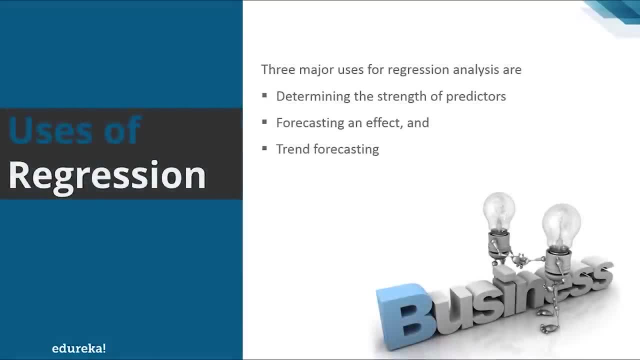 Well, there are major three uses of regression analysis, The first being determining the strength of predicators. The regression might be used to identify the strength of the effect that the independent variables have on the dependent variable. For example, you can ask question like: what is the strength of relationship between sales and marketing spending? 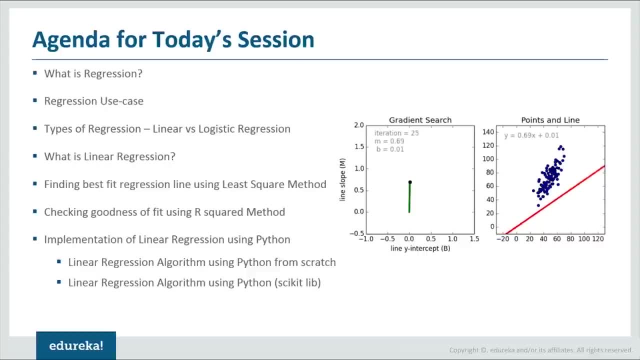 And then, finally, what we'll do will optimize it using the gradient descent method. In the last part, on the coding session, I'll teach you to implement linear regression using Python, And the coding session would be divided into two parts. The first part would consist of linear regression using Python from scratch. 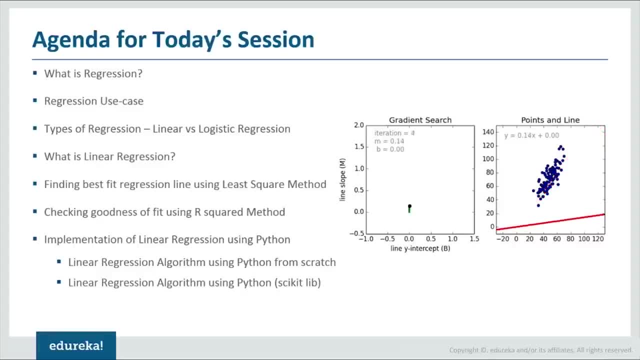 where you will use the mathematical algorithm that you have learned in this session. And in the next part of the coding session we'll be using scikit-learn for Derek implementation of linear regression. So let's begin our session with what is regression? 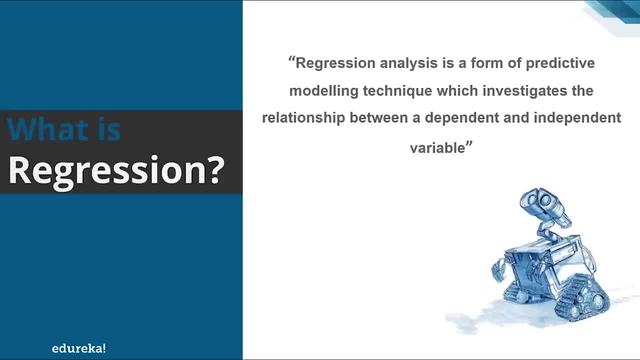 Well, regression analysis is a form of predictive modeling technique which investigates the relationship between a dependent and independent variable. A regression analysis involves graphing a line over a set of data points that most closely fits the overall shape of the data. A regression shows the changes in a dependent variable on the y-axis. 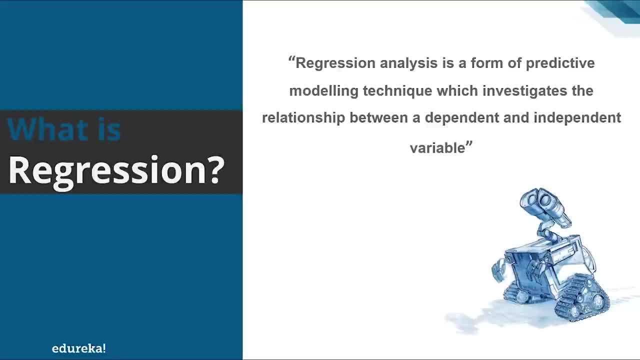 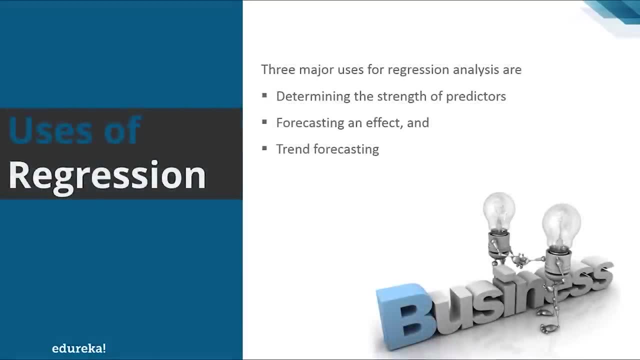 to the changes in the explanatory variable on the x-axis. Fine, Now you'd ask what are the uses of regression? Well, there are major three uses of regression analysis, The first being determining the strength of predicators. The regression might be used to identify the strength of the effect that the independent variables. 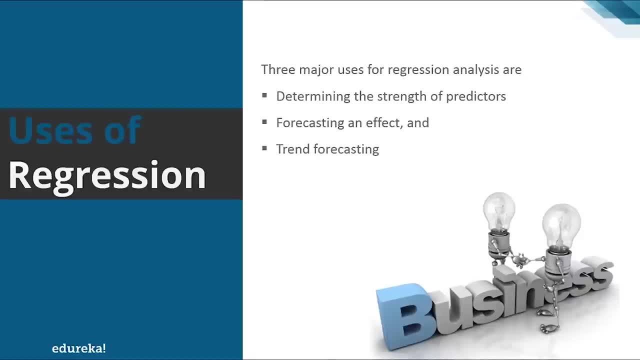 have on the dependent variable. For example, you can ask question like what is the strength of relationship between sales and marketing spending, or what is the relationship between age and income? second, is forecasting an effect in this? The regression can be used to forecast effects or impact of changes. 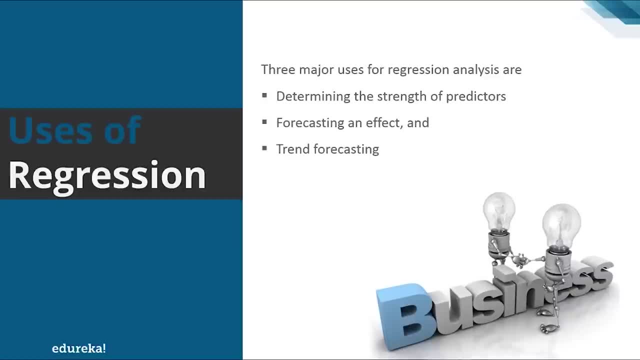 That is the regression analysis. help us to understand how much the dependent variable changes with the change in one or more independent variable. fine, For example, you can ask question like: how much additional sale income will I get for each thousand dollars spent on marketing? third is: 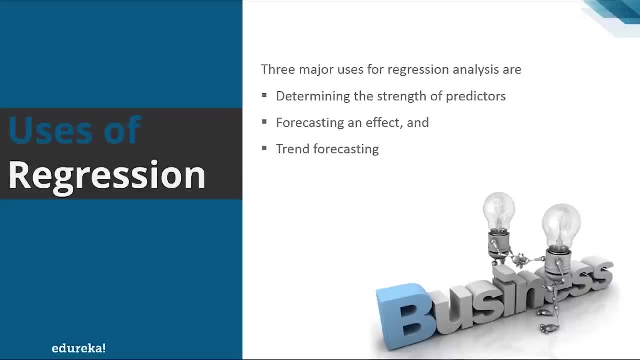 trend forecasting. in this, the regression analysis predict trends and future values. The regression analysis can be used to get point estimates. in this you can ask questions like what will be the price of Bitcoin in next six months, right? So next topic is linear versus logistic regression. by now, 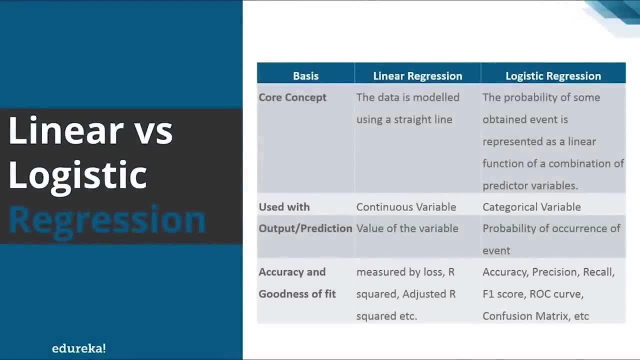 I hope that you know what a regression is, So let's move on and understand its type. So there are various kinds of regression, Like linear regression, logistic regression, polynomial regression and others. alright, but for this session will be focusing on linear and logistic regression. 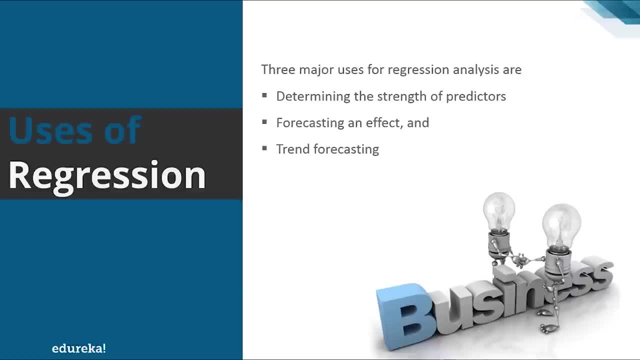 or what is the relationship between age and income? second, is forecasting an effect in this? the regression can be used to forecast effects or impact of changes. That is, the regression analysis help us to understand how much the dependent Variable changes with the change in one or more independent variable. 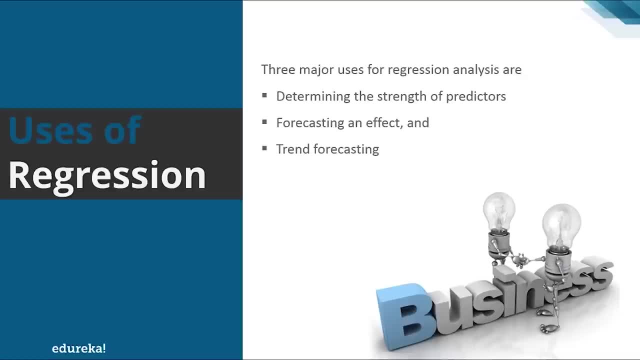 fine. For example, you can ask question like: how much additional sale income will I get for each thousand dollars spent on marketing? third is trend forecasting. in this, the regression analysis predict Trends and future values. the regression analysis can be used to get point estimates. in this, you can ask questions like: what will be the price of Bitcoin in next six months? 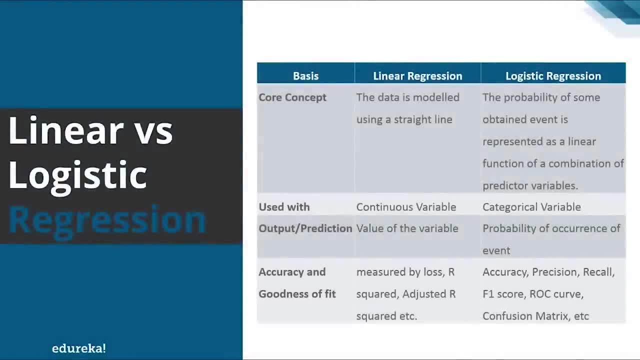 right. So next topic is linear versus logistic regression. By now I hope that you know what a regression is, So let's move on and understand its type. So there are various kinds of regression, like linear regression, logistic regression, polynomial regression and others. alright, 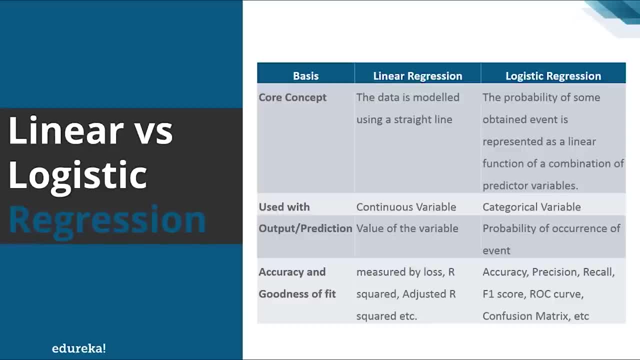 but for this session will be focusing on linear and logistic regression. So let's move on and let me tell you what is linear regression and what is logistic regression. Then what we'll do will compare both of them. Alright, so starting with linear regression in simple linear regression, 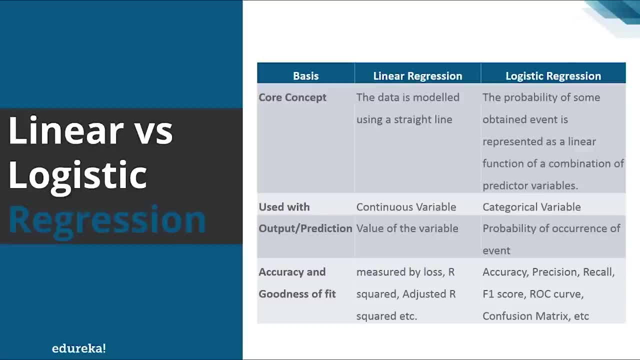 We are interested in things like: y equals Well MX plus C. So what we are trying to find is the correlation between X and Y variable. This means that every value of X has a corresponding value of Y in it If it is continuous. 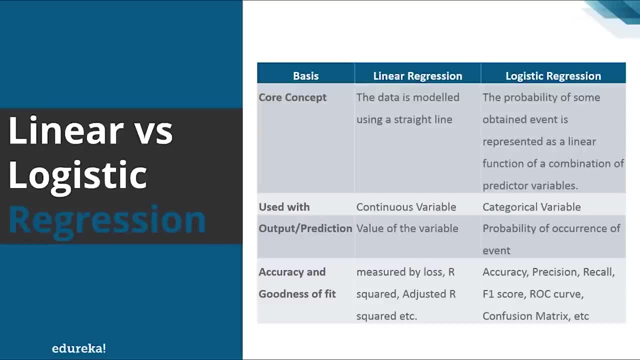 I like, however, and logistic regression. We are not fitting our data to a straight line like linear regression. Instead, what we are doing, We are mapping Y versus X to a sigmoid function. in logistic regression, What we find out is: is Y 1 or 0 for this particular value of X? 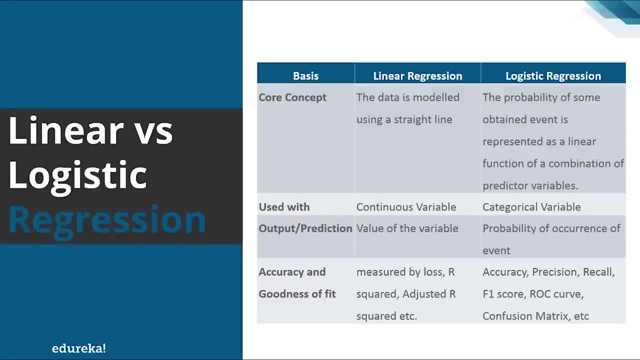 So this? we are essentially deciding true or false value for a given value of X. fine, So as a core concept of linear regression, you can say that the data is model using a straight line. We're in the case of logistic regression, The data is model using a sigmoid function. 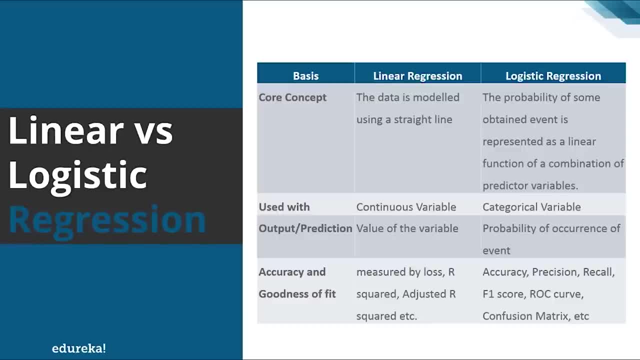 So let's move on and let me tell you what is linear regression and what is logistic regression. then what we'll do will compare both of them, Alright. so, starting with linear regression, in simple linear regression, We are interested in things like y equal MX plus C. 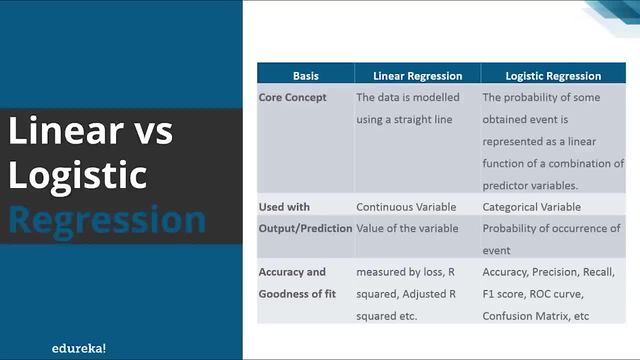 So what we are trying to find is the correlation between X and Y variable. This means that every value of X has a corresponding value of Y in it If it is continuous. I like, however, in logistic regression, we are not fitting our data to a straight line like linear regression instead. 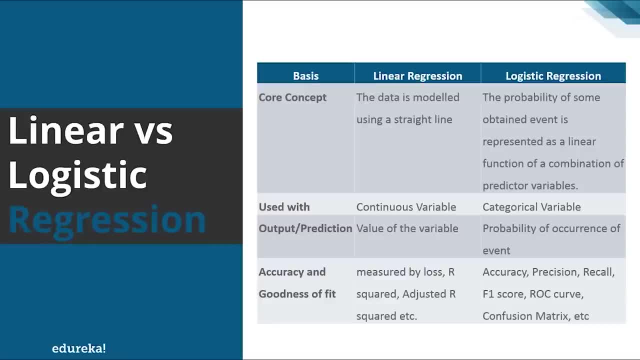 What we are doing? We are mapping Y versus X to a sigmoid function in logistic regression. What we find out is: is Y 1 or 0 for this particular value of X? So this: we are essentially deciding true or false value for a given value of X. fine, 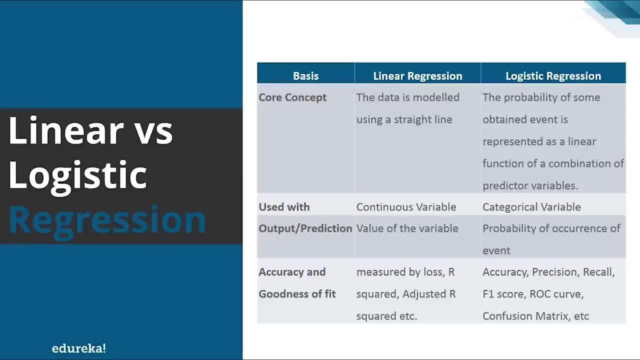 So, as a core concept of linear regression, you can say that the data is model using a straight line, where in the case of logistic regression, the data is model using a sigmoid function. The linear regression is used with continuous variables. On the other hand, the logistic regression, it is used with categorical variable. 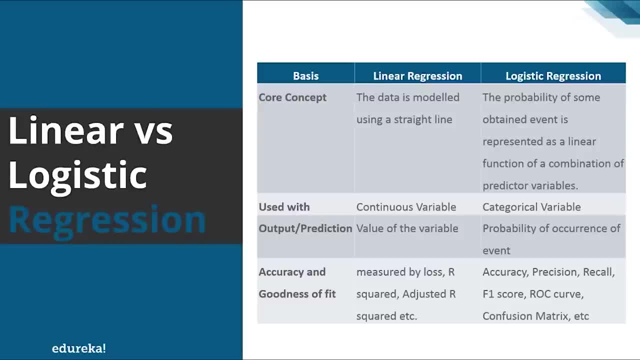 The output or the prediction of a linear regression is the value of the variable. On the other hand, the output of prediction of a logistic regression is the probability of occurrence of the event. Now how will you check the accuracy and goodness of fit in case of linear regression? 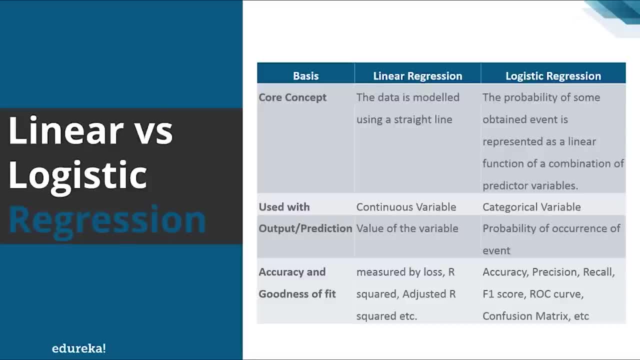 We have various methods, like measured by loss, R squared, adjusted R squared, Etc. While in the case of logistic regression you have accuracy, precision, recall, F1 score, which is nothing but the harmonic mean of precision and recall. Next is ROC curve for determining the probability threshold for classification. 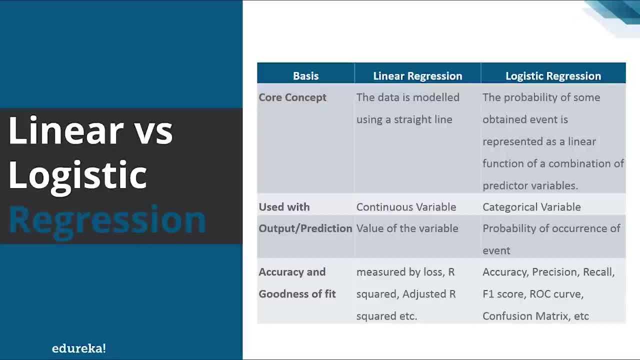 or the confusion, Matrix, Etc. There are many. alright, so, summarizing the difference between linear and logistic regression, You can say that the type of function you are mapping to is the main point of difference between linear and logistic regression. A linear regression Maps a continuous X to a continuous by, on the other hand, a logistic regression. 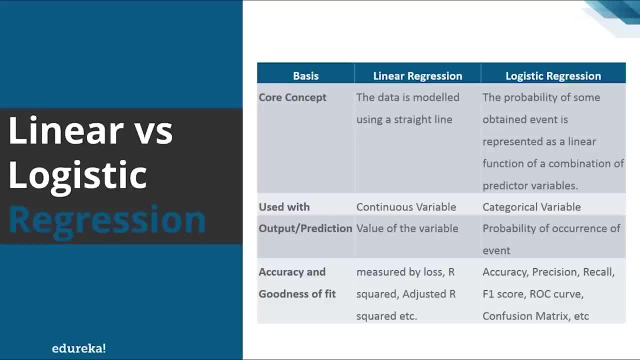 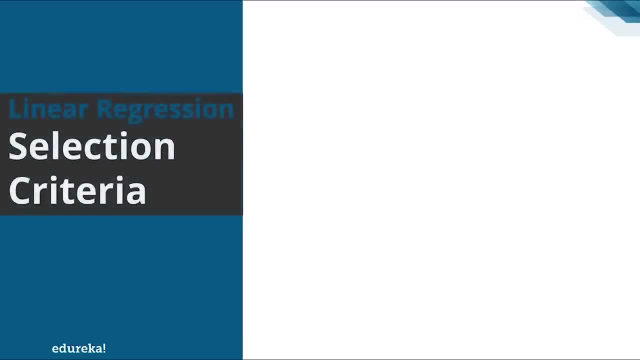 Maps a continuous X to the binary Y, So we can use logistic regression to make category or true-false decisions from the data. Fine, So let's move on ahead. Next is linear regression. selection criteria, or you can say when will you use linear regression. 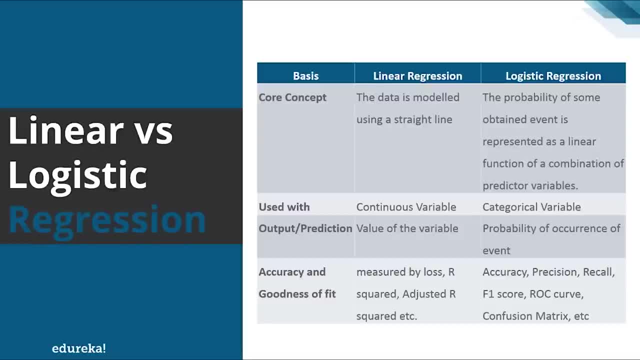 The linear regression is used with continuous variables. On the other hand, the logistic regression it is used with categorical variable. the output or the prediction of a linear regression is the value of the variable. on the other hand, the output of prediction of a logistic regression Is the probability of occurrence of the event. 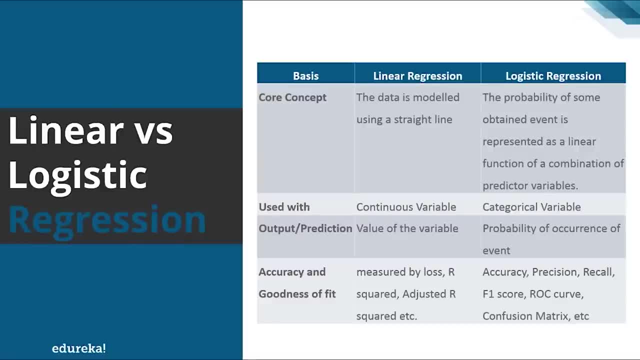 Now, how will you check the accuracy and goodness of fit? in case of linear regression, You have various methods like measured by loss, R squared, adjusted R squared, Etc. While in the case of logistic regression, you have accuracy, precision, recall, F1 score, which is nothing but the harmonic mean of precision and recall. next is ROC curve for determining. 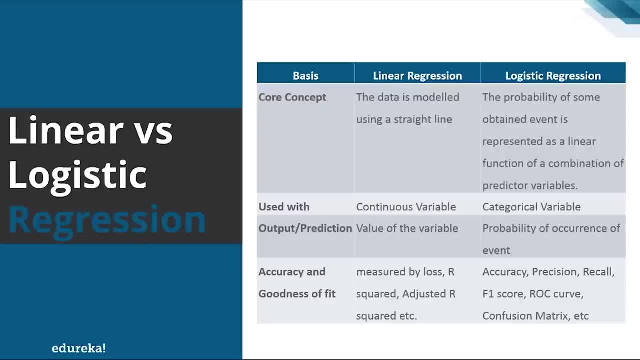 the probability threshold for classification, or the confusion Matrix, Etc. There are many, all right. So, summarizing the difference between linear and logistic regression, You can say that the type of function you are mapping to is the main point of difference between linear and logistic regression. a linear regression maps a continuous X to a continuous. 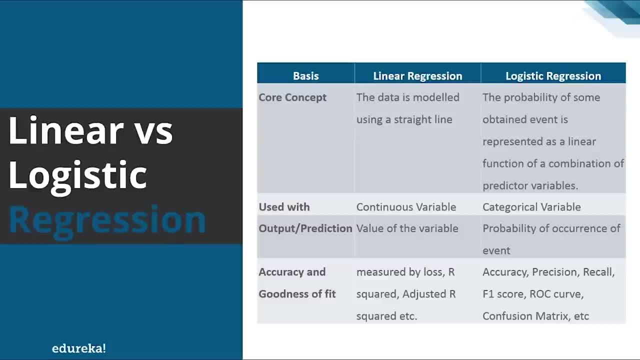 by. on the other hand, a logistic regression maps a continuous X to the binary Y, so we can use logistic regression to make category or true-false decisions from the data. fine, So let's move on ahead. next is linear regression selection criteria. or you can say: 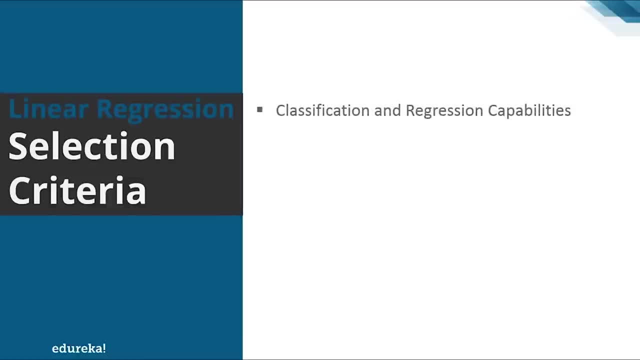 when will you use linear regression? So the first is classification and regression capabilities. regression models predict a continuous variable, such as the sales made on a day, or predict the temperature of a city. their reliance on a polynomial, like a straight line, to fit a data set poses a real challenge when it comes towards. 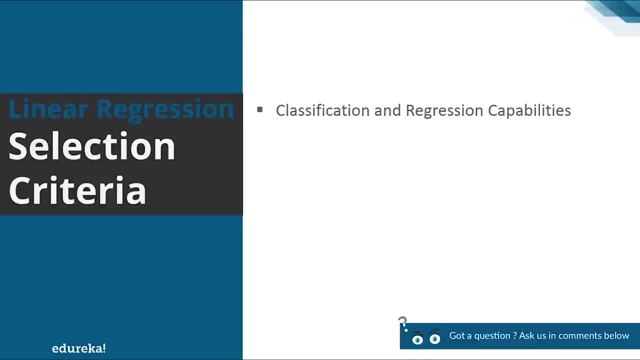 building a classification capability. Let's imagine that you fit a line with the training points that you have. now imagine you add some more data points to it. But in order to fit it, what do you have to do? You have to change your existing model. 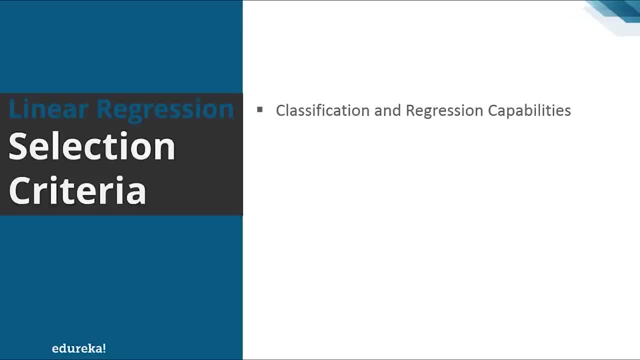 That is, maybe you have to change the threshold itself. So this will happen with each new data point you add to the model. Hence the linear regression is not good for classification models, Fine. Next is data quality. each missing value removes one data point that could optimize the regression. 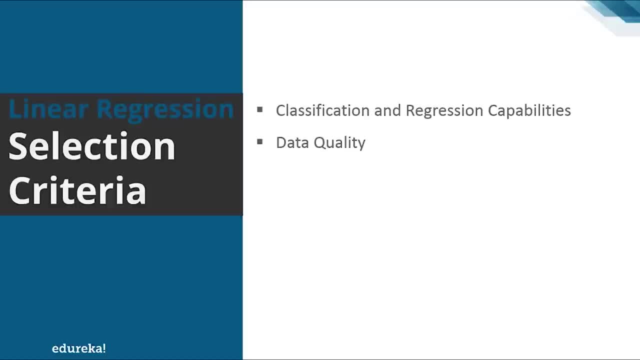 and simple linear regression. The outliers can significantly disrupt the outcome. just for now, You can know that if you remove the outliers, your model will become very good, All right. So this is what data quality. next is computational complexity. The linear regression is often not computationally expensive as compared. 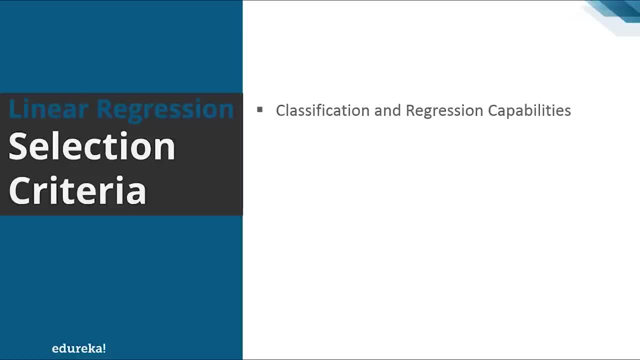 So the first is classification and regression capabilities. regression models predict a continuous variable, Such as the sales made on a day or predict the temperature of a city. Their reliance on a polynomial, like a straight line, to fit a data set poses a real challenge when it 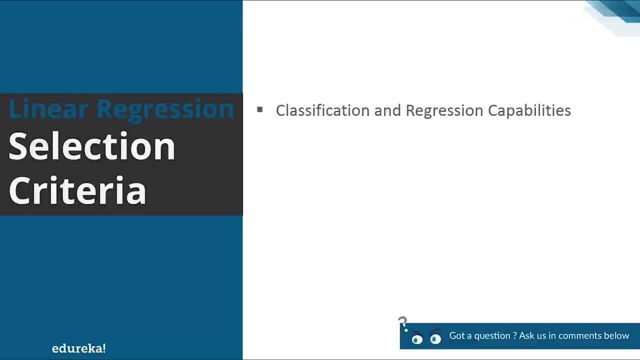 comes towards building a classification capability. Let's imagine that you fit a line with the training points that you have. now imagine you add some more data points to it. But in order to fit it, what do you have to do? You have to change your existing model. that is, maybe you have to change the threshold itself. 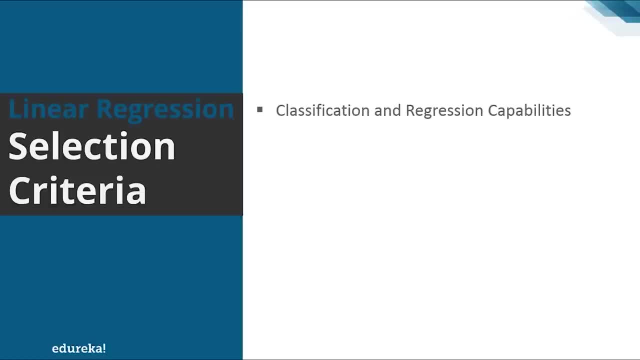 So this will happen. with each new data point you are to the model, Hence The linear regression is not going to change. It's good for classification models, Fine. Next is data quality. each missing value removes one data point that could optimize the regression. 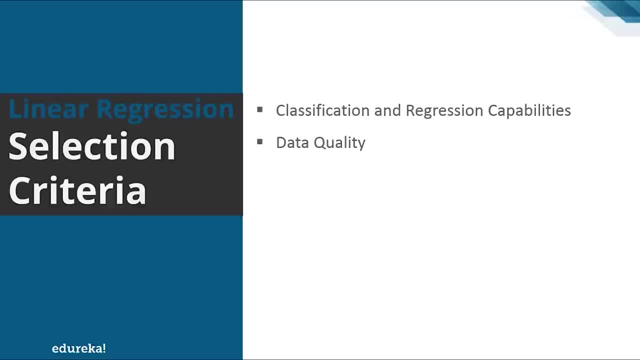 and simple linear regression, The outliers can significantly disrupt the outcome. just for now, You can know that if you remove the outliers, your model will become very good, All right. So this is what: data quality. next is computational complexity. A linear regression is often not computationally expensive as compared to the decision tree. 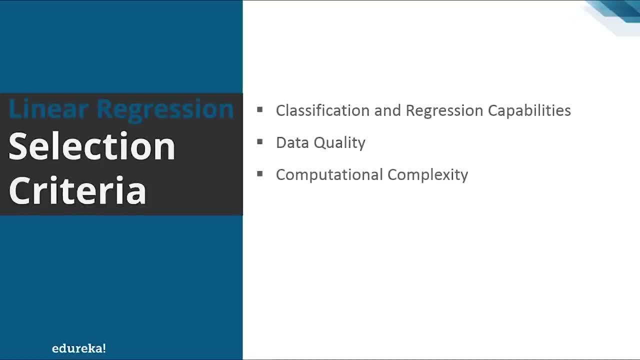 or the clustering algorithm. the order of complexity for n training examples And X features usually falls in either bigger of x square or bigger of X in next is comprehensible and transparent. the linear regression are easily comprehensible and transparent in nature. They can be represented by a simpler mathematical notation to anyone and can be understood very easily. 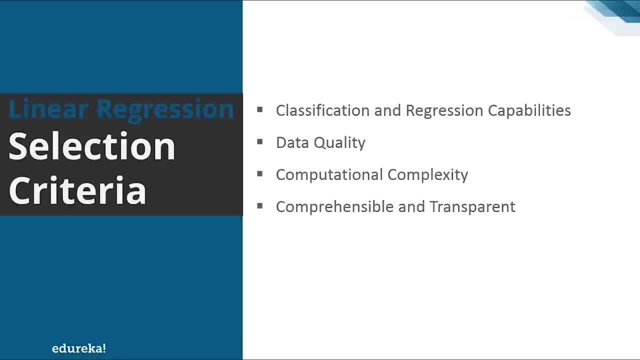 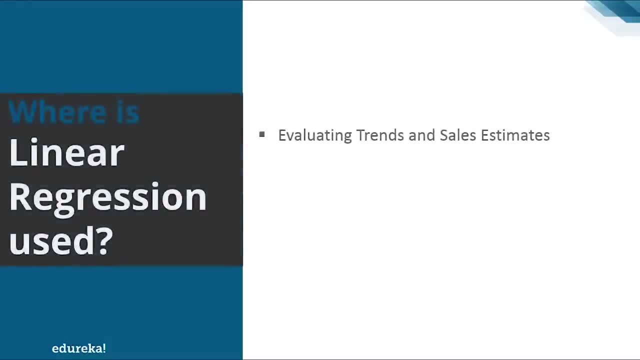 So these are some of the criteria based on which you will select the linear regression algorithm. All right. next is: where is linear regression used? first is evaluating Trends and sales estimate. Well, linear regression can be used in business to evaluate Trends and make estimates of forecasts. 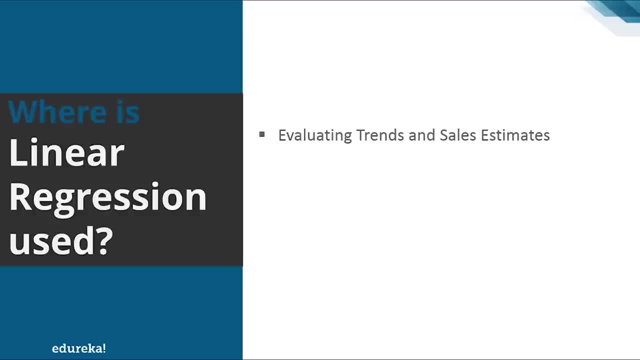 For example, if a company sale have increased steadily every month for past few years, then conducting a linear analysis on the sales data, with monthly sales on the y-axis and time on the x-axis, This will give you a line that predicts the upward Trends in the sale. after creating the trend line, 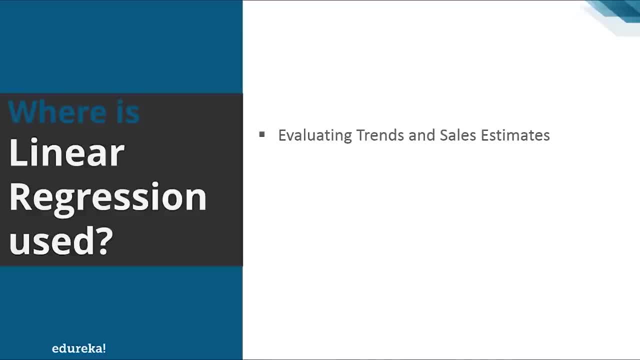 The company could use the slope of the lines to forecast sale in future months. Next is analyzing the impact of price changes. Well, linear regression can be used to analyze the effect of pricing on consumer behavior. For instance, if a company changes the price on a certain product several times, then it can record the quantity itself. 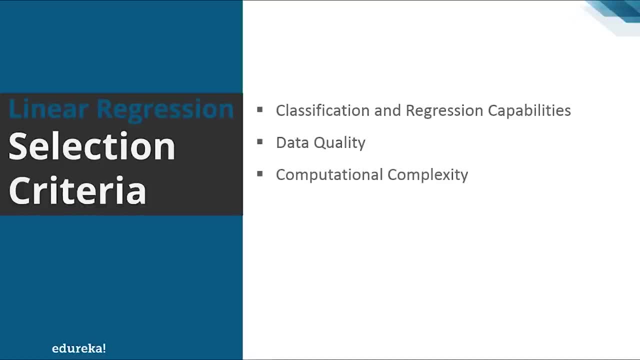 to the decision tree or the clustering algorithm. the order of complexity for n training, example, and X features usually falls in either big O of X square or big O of X. n next is comprehensible and transparent. the linear regression are easily comprehensible and transparent in nature. 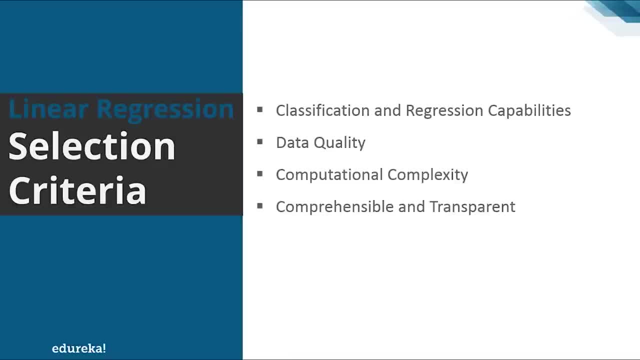 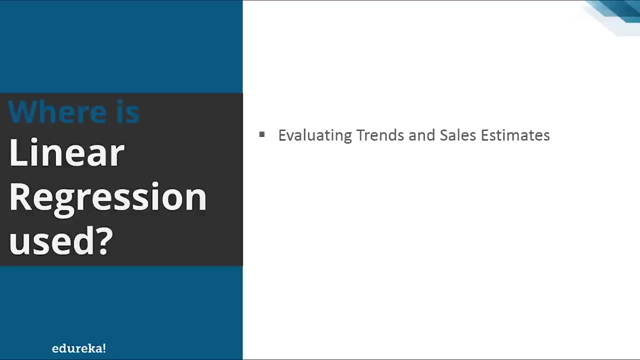 They can be represented by a simpler mathematical notation to anyone and can be understood very easily. So these are some of the criteria based on which you will select the linear regression algorithm. All right. next is: where is linear regression used? first is evaluating Trends and sales estimate. well, linear aggression can be used in business to evaluate Trends. 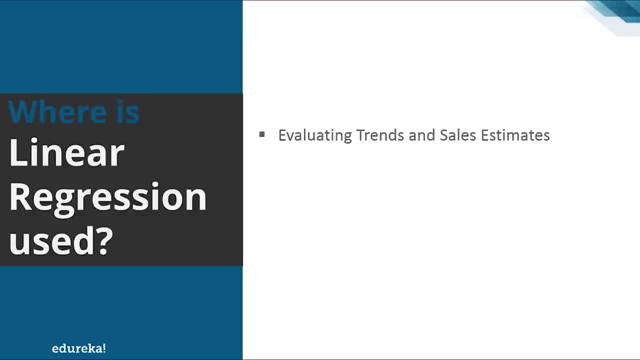 and make estimates of forecasts. For example, if a company sale have increased steadily every month for past few years, then conducting a linear analysis on the sales data with monthly sales on the y-axis and time on the x-axis, This will give you a line that predicts the upward Trends. 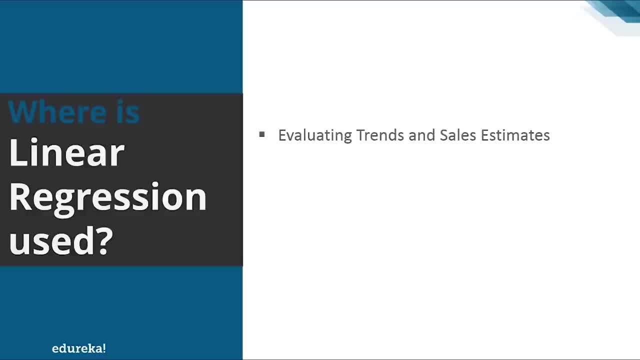 in the sale. after creating the Trend line, the company could use the slope of the lines to forecast sale in future months. next is analyzing the impact of price changes. Well, linear regression can be used to analyze the effect of pricing on consumer behavior. For instance, if a company changes the price on a certain product several times. 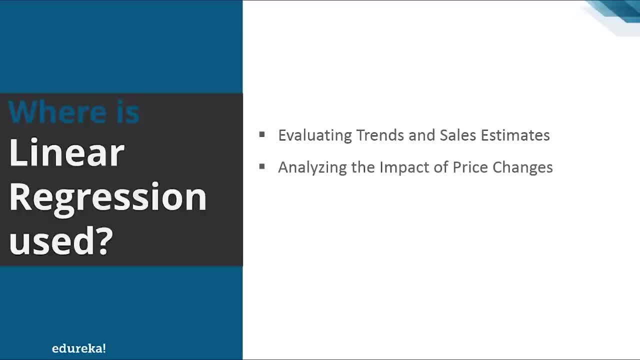 then it can record the quantity itself for each price level and then perform a linear regression with sole quantity as a dependent variable and price as the independent variable. this would result in a line that depicts the extent to which the customer reduce their consumption of the product as the price is increasing. 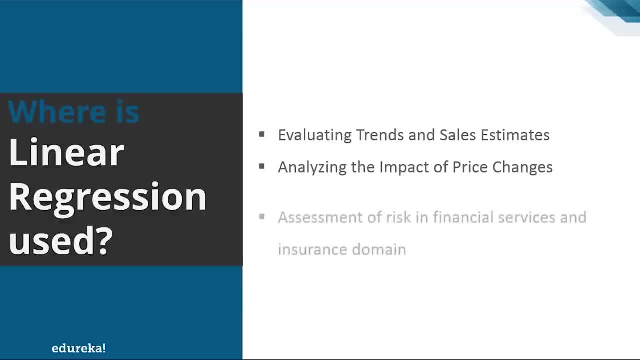 So this result would help us in future pricing decisions. Next is assessment of risk in financial services and insurance domain. Well, linear regression can be used to analyze the risk. For example, a health insurance company might conduct a linear regression algorithm. how it can do? it can do it by plotting the number of claims per customer against its age. 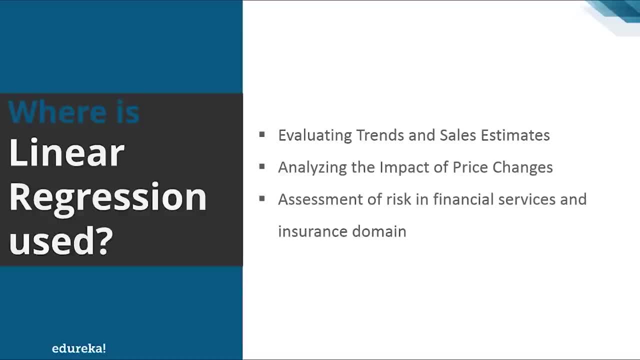 and they might discover that the old customers tend to make more health insurance claims. Well, the result of such an analysis might guide important business decisions. All right, So by now you have just a rough idea of what linear regression algorithm is like, what it does, where it is used, when you should use it. 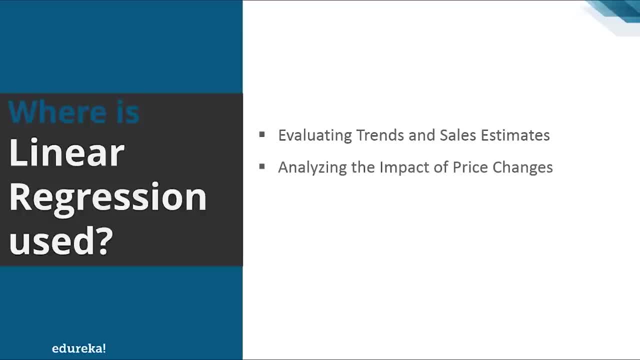 for each price level and then perform a linear regression, with sole quantity as a dependent variable and price as the independent variable. this would result in a line that depicts the extent to which the customer reduce their consumption of the product as the price is increasing. So this result would help us in future pricing decisions. 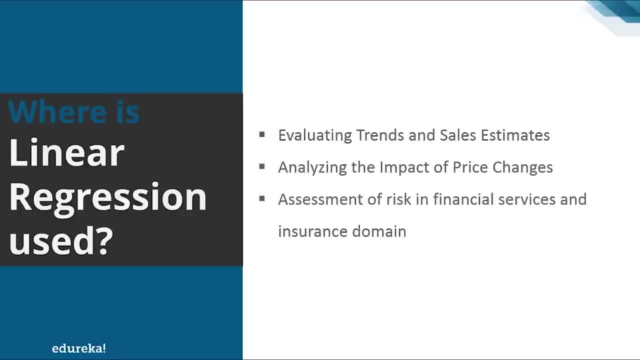 Next is assessment of risk in financial services and insurance domain. Well, linear regression can be used to analyze the risk. For example, a health insurance company might conduct a linear regression algorithm. how it can do it can do it by plotting the number of claims per customer against its age. 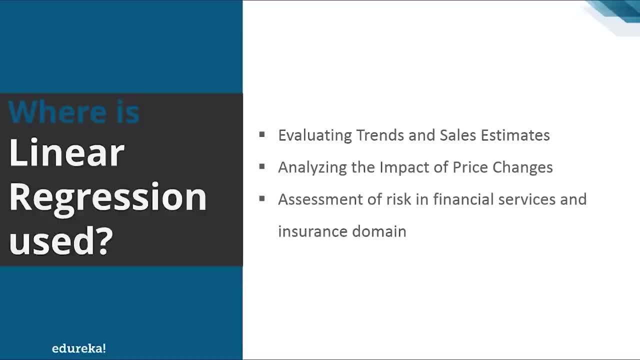 and they might discover that the old customers tend to make more health insurance claim. Well, the result of such an analysis might guide important business decisions. All right, So by now you have just a rough idea of What linear regression algorithm is like, what it does. 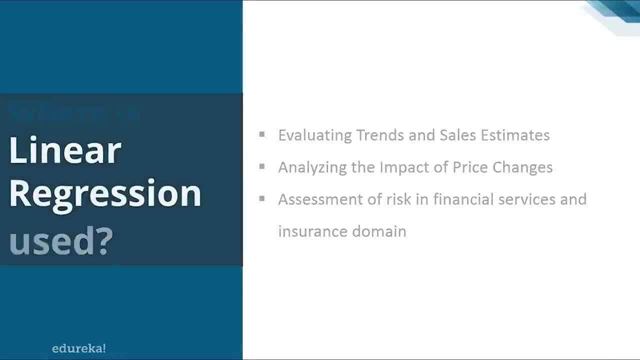 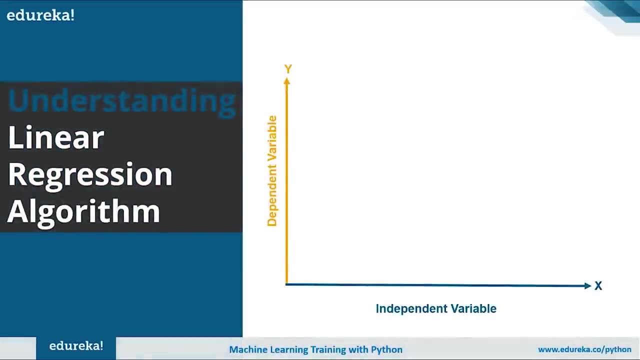 where it is used, when you should use it. All right, Now let's move on and understand the algorithm in depth. So suppose you have independent variable on the x-axis and dependent variable on the y-axis. All right, Suppose this is the data point on the x-axis. 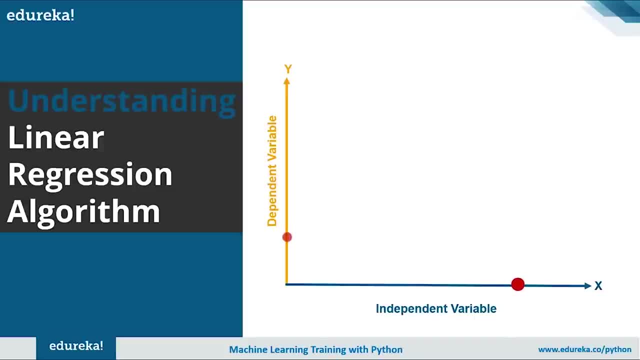 the independent variable is increasing on the x-axis and so does the dependent variable on the y-axis. So what kind of linear regression line you would get? you'd get a positive linear regression line, All right, As the slope would be positive. next is suppose you have an independent variable. 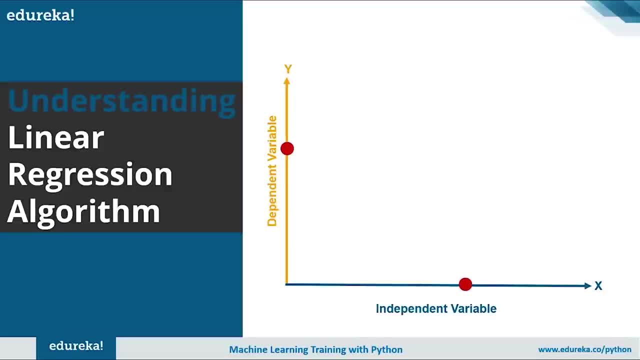 on the x-axis, which is increasing, and, on the other hand, the dependent variable on the y-axis, that is decreasing. So what kind of line will you get in that case? You will get a negative regression line in this case, as the slope of the line is negative. 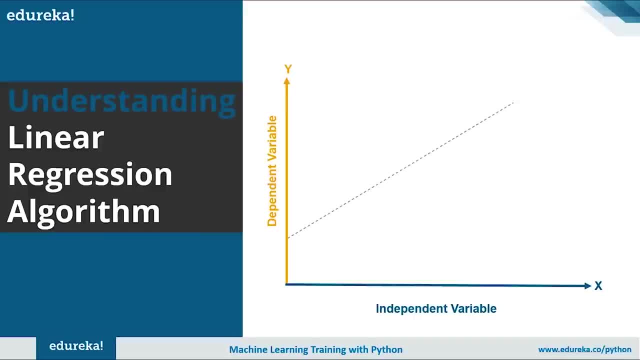 and this particular line, that is, line of y equal MX plus C, is a line of linear regression which shows the relationship between independent variable and dependent variable, and this line is only known as line of linear regression. Okay, so let's add some data points to our graph. 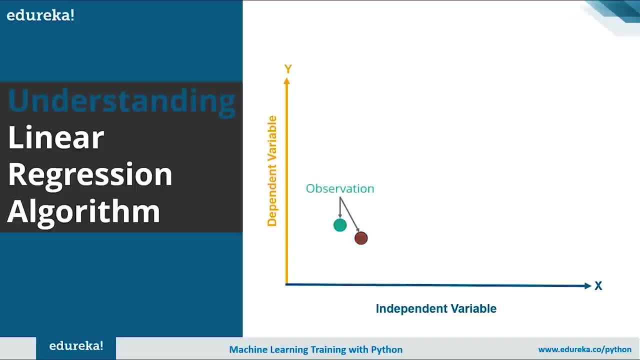 So these are some observation or data points on our graphs. Let's plot some more. Okay, Now, all our data points are plotted. now our task is to create a regression line, or the best fit line. All right, Now, once our regression line is drawn, now 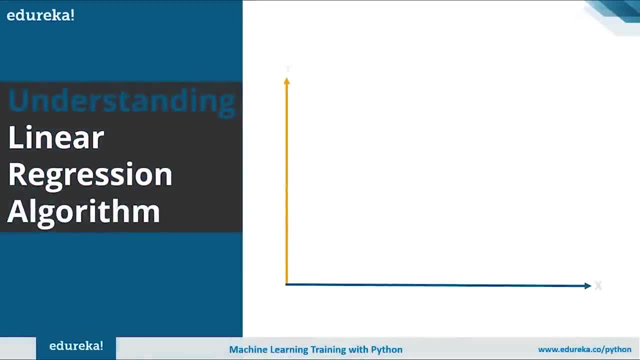 All right, Now let's move on and understand the algorithm in depth. So suppose you have independent variable on the x-axis and dependent variable on the y-axis. All right, Suppose this is the data point on the x-axis. The independent variable is increasing on the x-axis. 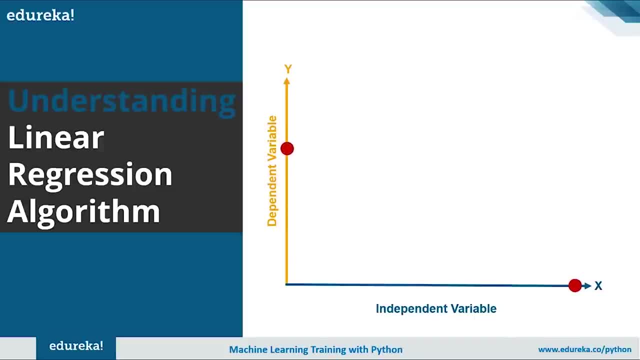 And so does the dependent variable on the y-axis. So what kind of linear regression line you would get? you'd get a positive linear regression line, All right, as the slope would be positive. next is suppose you have an independent variable on the x-axis which is increasing, and on the other hand, 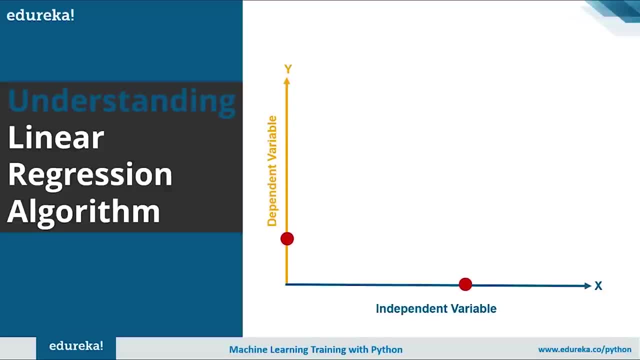 the dependent variable on the y-axis that is decreasing. So what kind of line will you get in that case? You will get a negative regression line in this case, as the slope of the line is negative, and this particular line, that is, line of y equal MX plus C. 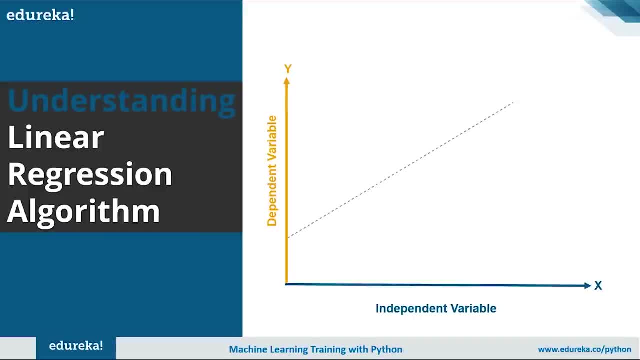 Is a line of linear regression which shows the relationship between independent variable and dependent variable, and this line is only known as line of linear regression. Okay, So let's add some data points to our graph. So these are some observation or data points on our graphs. 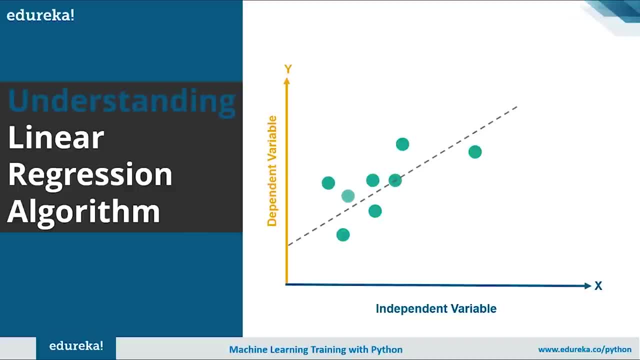 Let's plot some more. Okay, Now all our data points are plotted. Now our task is to create a regression line, or the best fit line. All right, Now, once our regression line is drawn, now it's the task of prediction. Now, suppose this is our estimated value. 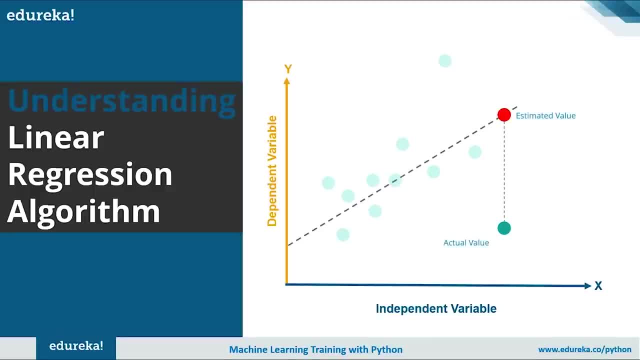 or the predicted value, and this is our actual value. Okay, So what we have to do, our main goal, is to reduce this error, that is, to reduce the distance between the estimated or the predicted value and the actual value. The best fit line would be the one which had the least error. 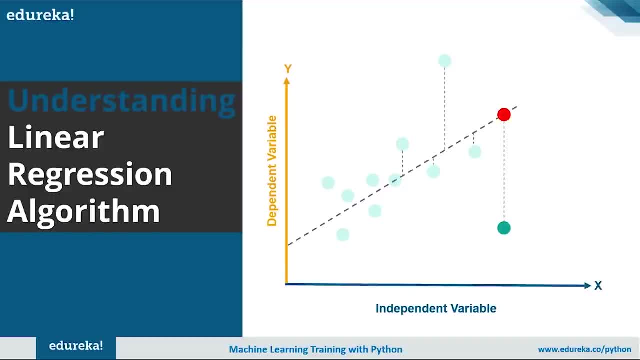 or the least difference in estimated value and the actual value. All right, In other words, we have to minimize the error. This was a brief understanding of linear regression algorithm. Soon We'll jump to its mathematical implementation, But for then, let me tell you this. 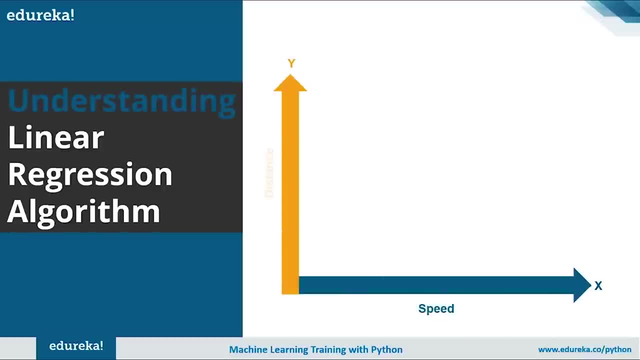 Suppose you draw a graph with speed on the x-axis and distance covered on the y-axis, with the time remaining constant. If you plot a graph between the speed traveled by the vehicle and the distance traveled in a fixed unit of time, then you will get a positive relationship. 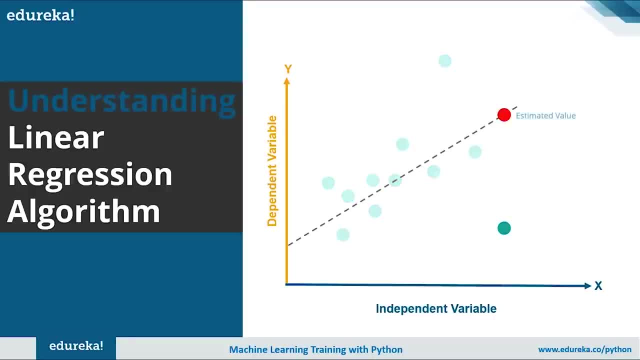 it's the task of prediction. Now suppose this is our estimated value or the predicted value, and there's our actual value. Okay, So what we have to do? Our main goal, is to reduce this error, that is, to reduce the distance between the estimated or the predicted value. 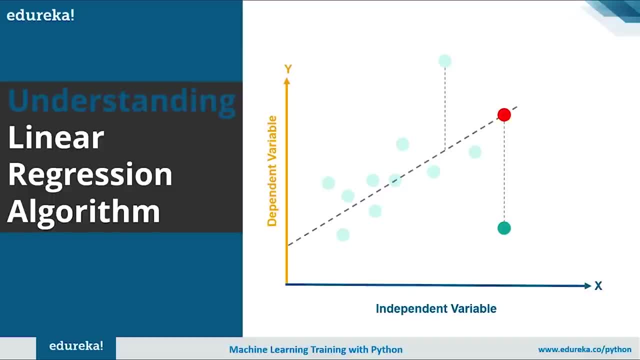 and the actual value. The best fit line would be the one which had the least error or the least difference in estimated value and the actual value. All right, In other words, we have to minimize the error. This was a brief understanding of linear regression algorithm. 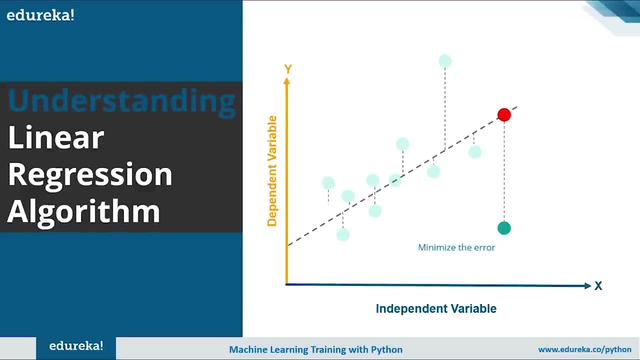 soon We'll jump to its mathematical implementation, But for then let me tell you this: suppose you draw a graph with speed on the x-axis and distance covered on the y-axis, with the time remaining constant. If you plot a graph between the speed traveled by the vehicle, 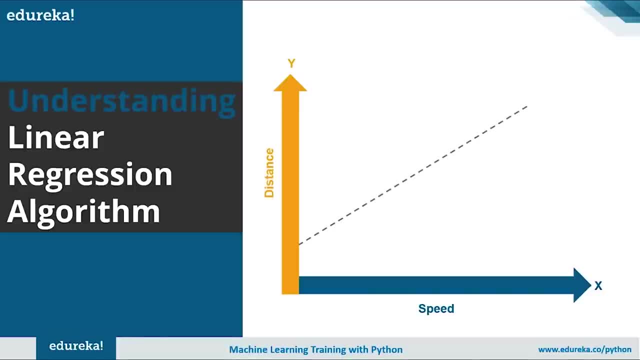 and the distance traveled in a fixed unit of time, then you will get a positive relationship, All right. So suppose the equation of line is y equal MX plus C, then in this case, why is the distance traveled in a fixed duration of time? X is the speed. 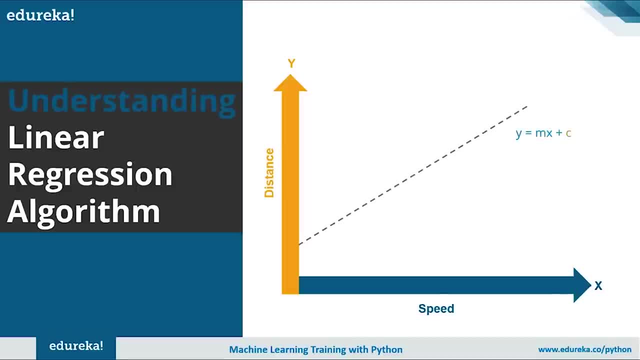 of vehicle. M is the positive slope of the line and C is the y intercept of the line. All right, Suppose the distance remaining constant. You have to plot a graph between the speed of the vehicle and the time taken to travel a fixed distance. that, in that case, 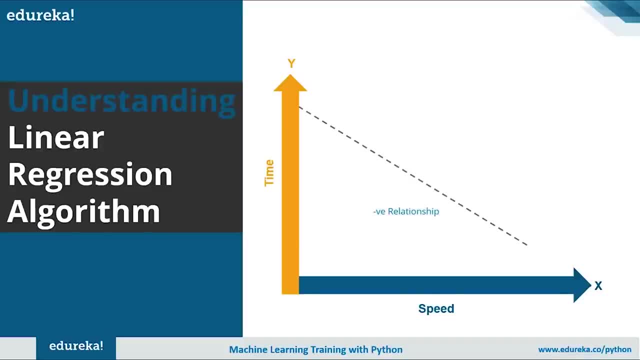 you will get a line with a negative relationship. All right, the slope of the line is negative. here The equation of line changes to y, equal minus of MX plus C, where Y is the time taken to travel a fixed distance, X is the speed of vehicle, M is the negative slope of the line and C is the y. 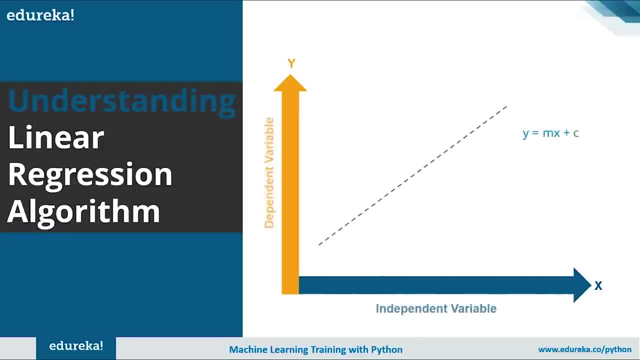 intercept of the line. All right, Now let's get back to our independent and dependent variable. So, in that term, Y is our dependent variable and X, that is our independent variable. Now let's move on and see the mathematical implementation of. 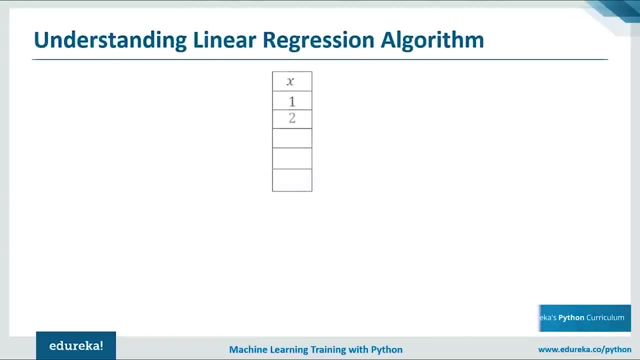 the things All right. So we have X equal 1, 2, 3, 4, 5.. Let's plot them on the x-axis, So 0, 1, 2, 3, 4, 5, 6.. All right, and we have Y as 3, 4, 2, 4, 5.. 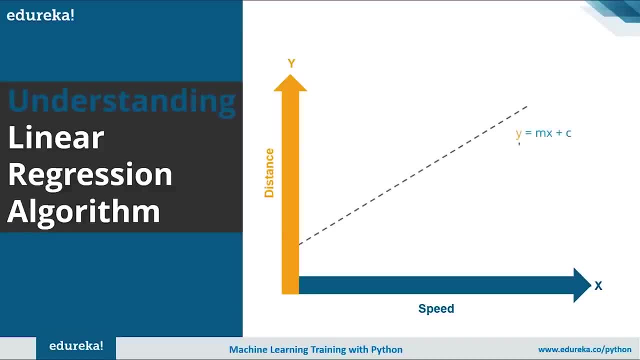 All right, So suppose the equation of line is y equal MX plus C. Then in this case, why is the distance traveled in a fixed duration of time? X is the speed of vehicle, M is the positive slope of the line and C is the y-intercept of the line. 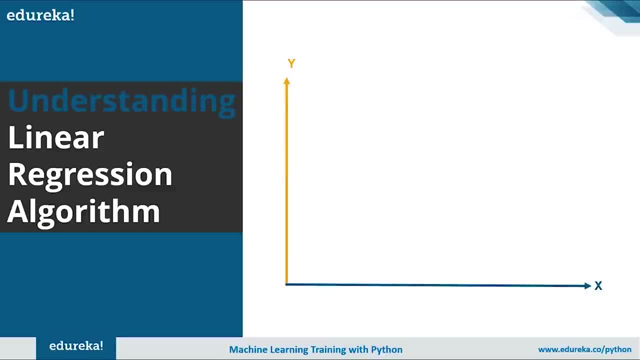 All right, suppose the distance remaining constant, You have to plot a graph between the speed of the vehicle and the time taken to travel a fixed distance. Then in that case you will get a line with a negative relationship. All right, the slope of the line is negative here. 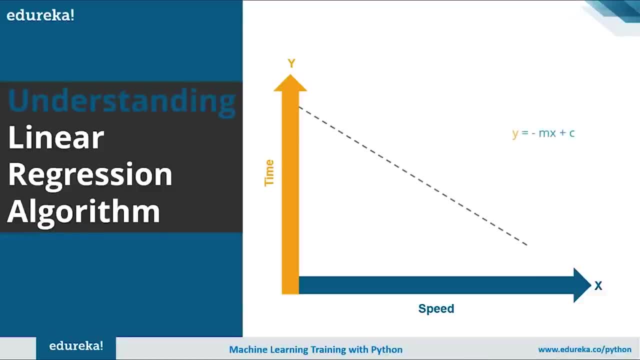 The equation of line changes to: y equal minus of MX plus C, Where y is the time taken to travel a fixed distance, X is the speed of vehicle, M is the negative slope of the line and C is the y-intercept of the line. 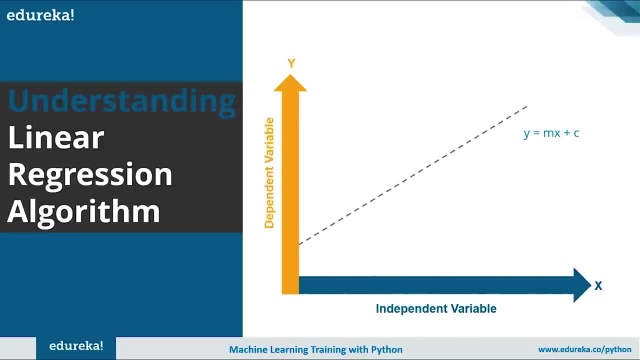 All right, Now let's get back to our independent and dependent variable. So, in that term, Y is our dependent variable and X that is our independent variable. Now let's move on and see the mathematical implementation of the things. All right, 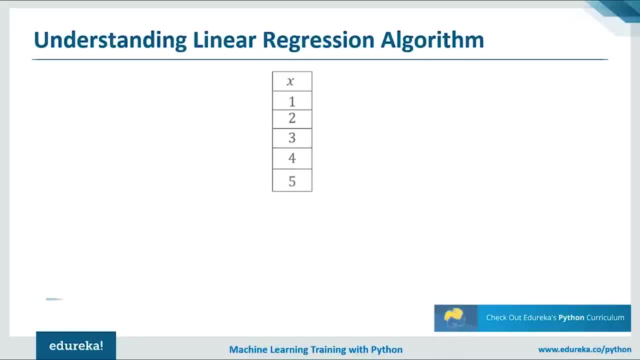 So we have x equal 1, 2, 3, 4, 5.. Let's plot them on the x-axis, So 0, 1, 2, 3, 4, 5, 6.. All right, and we have y as 3, 4, 2, 4, 5.. 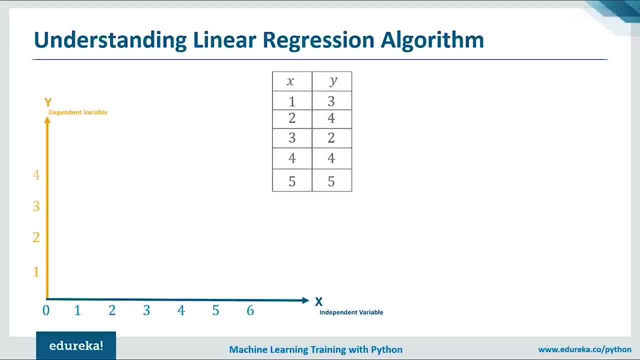 All right. So let's plot 1, 2, 3, 4, 5 on the y-axis. Now let's plot our coordinates one by one, So x equal 1 and y equal 3.. So we have here x equal 1 and y equal 3.. 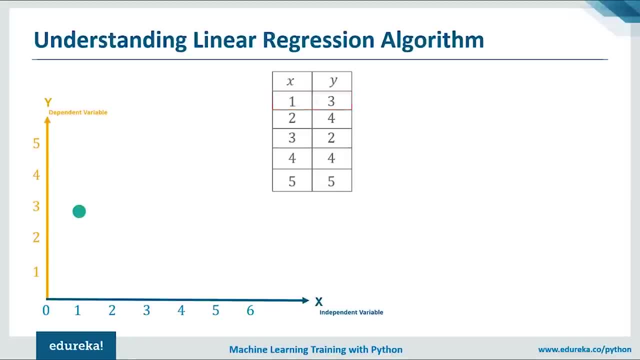 So this is our point 1, comma 3.. So, similarly, we have 1, 3, 2, 4, 3, 2, 4, 4 and 5, 5.. All right, So, moving on ahead, let's calculate the mean of x and y and plot it on the graph. 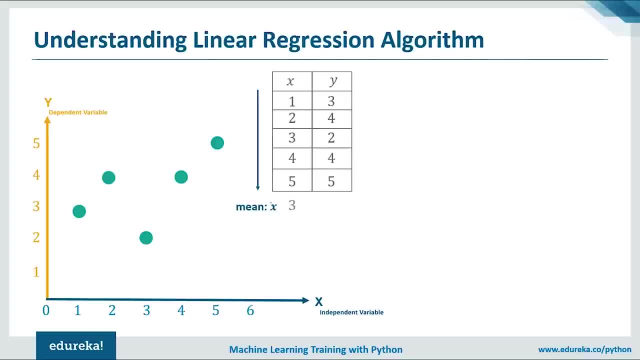 All right. So mean of X is 1 plus 2 plus 3 plus 4 plus 5.. 5 divided by 5, that is 3.. All right. Similarly, mean of Y is 3 plus 4 plus 2 plus 4 plus 5, that is 18.. 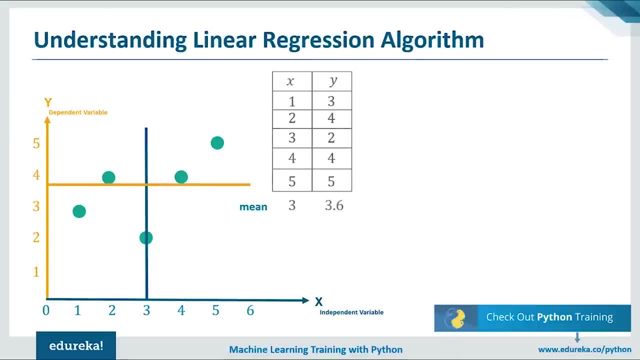 So 18 divided by 5, that is nothing but 3.6.. All right, So next, what we'll do will plot our mean, that is 3 comma 3.6, on the graph. Okay, so there's a point, 3 comma 3.6.. 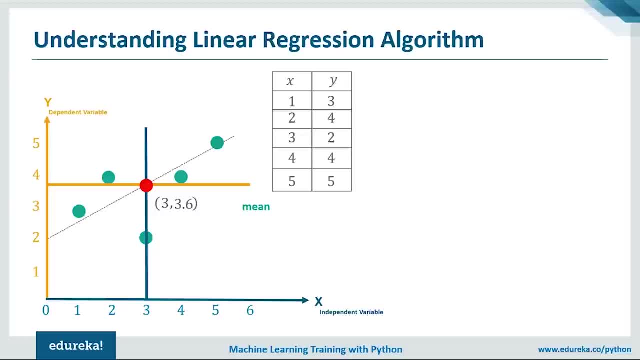 See, our goal is to find or predict the best fit line using the least square method. All right. So in order to find that, we first need to find the equation of line. So let's find the equation of our regression line, All right? 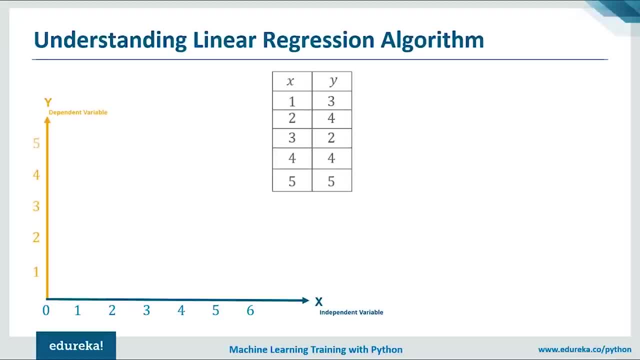 All right. So let's plot 1, 2, 3, 4, 5 on the y-axis. Now let's plot our coordinates one by one, So X equal 1 and y equal 3.. So we have here X equal 1 and y equal 3.. 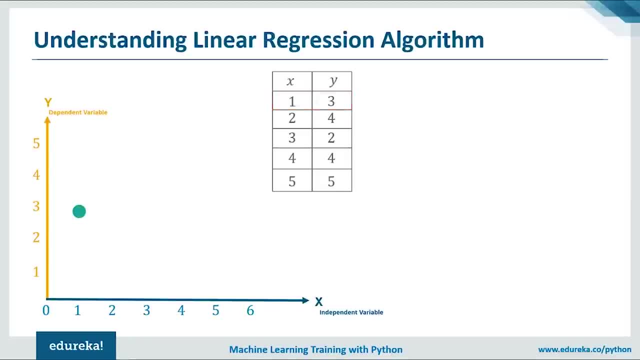 So this is our point 1, comma 3.. So, similarly, we have 1, 3, 2, 4, 3, 2, 4, 4 and 5, 5.. All right, So, moving on ahead, Let's calculate the mean of X and Y and plot it on the graph. 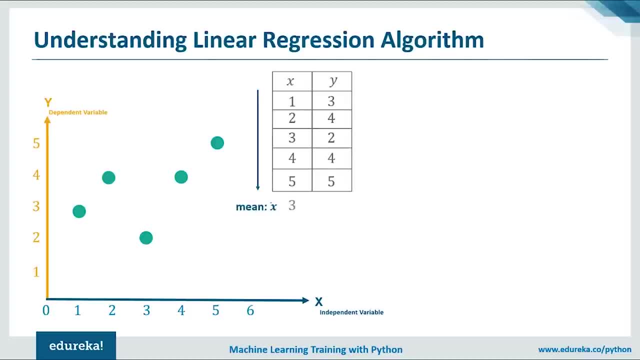 All right. So mean of X is 1 plus 2 plus 3 plus 4 plus 5 divided by 5.. That is 3.. All right. Similarly, mean of Y is 3 plus 4 plus 2 plus 4 plus 5.. 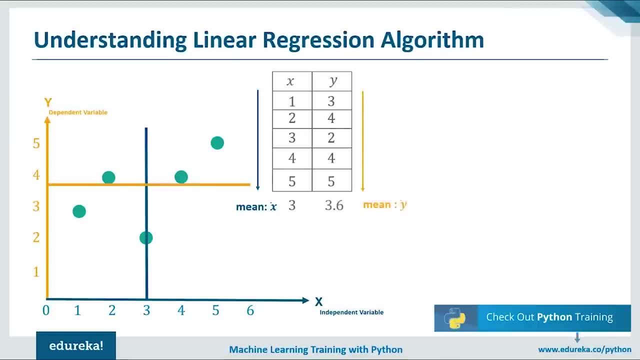 That is 18.. So 18 divided by 5, that is nothing but 3.6.. All right, So next what we'll do will plot our mean. that is 3 comma 3.6 on the graph. Okay, So there's a point 3 comma 3.6.. 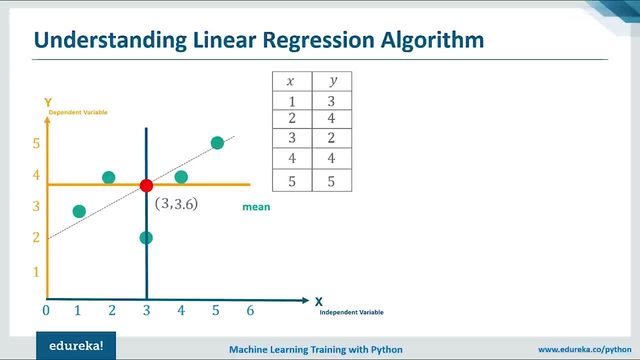 See, our goal is to find or predict the best fit line using the least square method. All right. So in order to find that, we first need to find the equation of line. So let's find the equation of our regression line, All right? 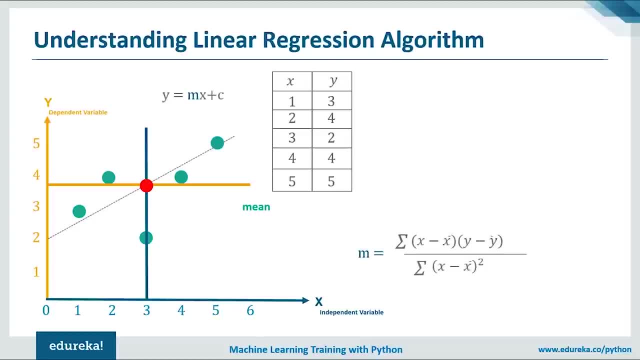 So let's suppose this is our regression line. Why? Why does it equal MX plus C? Now we have a equation of line, So all we need to do is find the value of M and C, where M equals summation of X minus X bar, multiplied by Y minus Y bar. 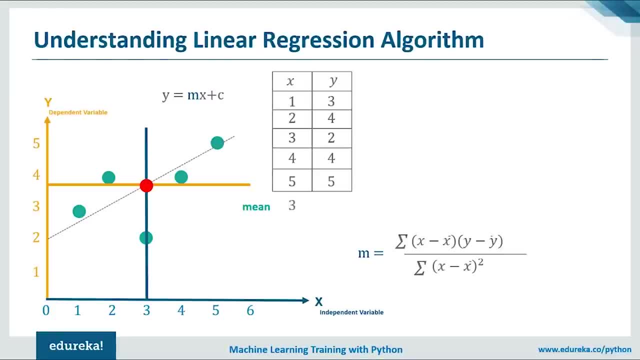 upon the summation of X minus X bar whole square. Don't get confused. Let me resolve it for you, All right. So, moving on ahead as a part of formula, what we are going to do will calculate X minus X bar. So we have X as 1 minus X bar as 3.. 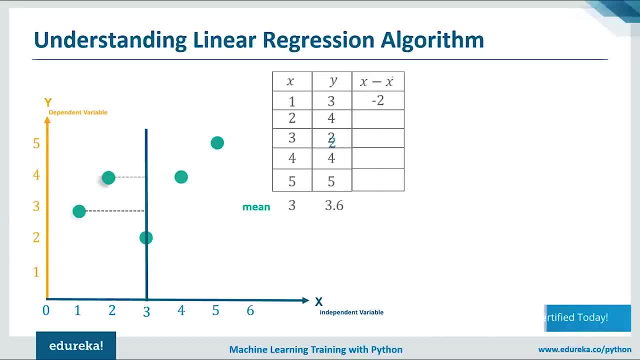 So 1 minus 3, that is minus 2.. Next we have X equal to minus its mean, 3, that is minus 1.. Similarly, We have 3 minus 3, 0, 4 minus 3, 1, 5 minus 3, 2.. 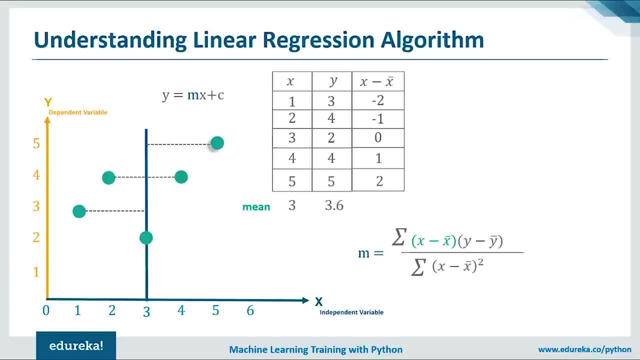 All right. So X minus X bar, It's nothing but the distance of all the point through the line Y, equal 3.. And what does this Y minus Y bar implies? it implies the distance of all the point from the line X, equal 3.6. fine, 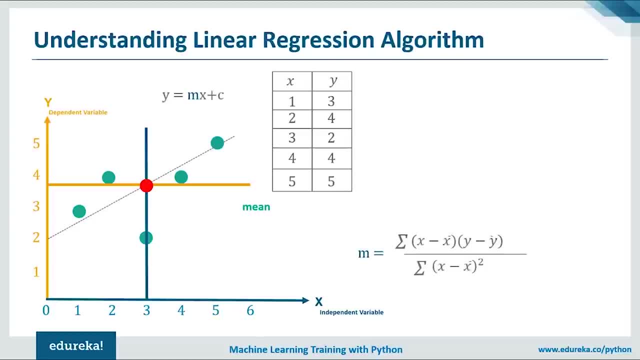 So let's suppose this is our regression line: y equal mx plus C. Now we have a equation of line, So all we need to do is find the value of m and C, where m equals summation of x minus x bar, multiplied by y minus y bar. 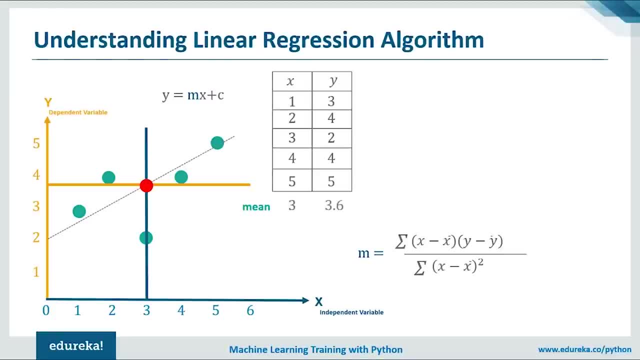 upon the summation of x minus x bar whole square. Don't get confused. Let me resolve it for you, All right. So, moving on ahead as a part of formula, what we are going to do will calculate x minus x bar. So we have x as 1 minus x bar as 3.. 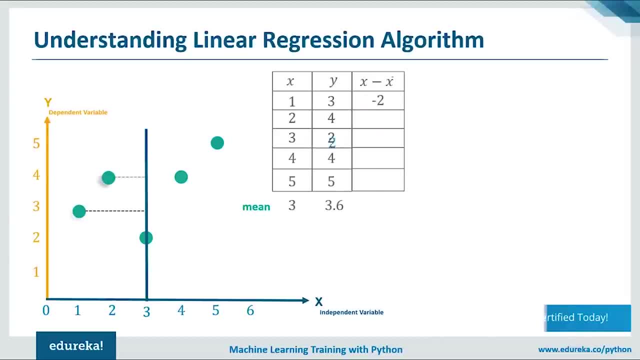 So 1 minus 3, that is minus 2. next We have x equal to minus its mean, 3, that is minus 1.. Similarly, We have 3 minus 3, 0, 4 minus 3, 1, 5 minus 3, 2.. 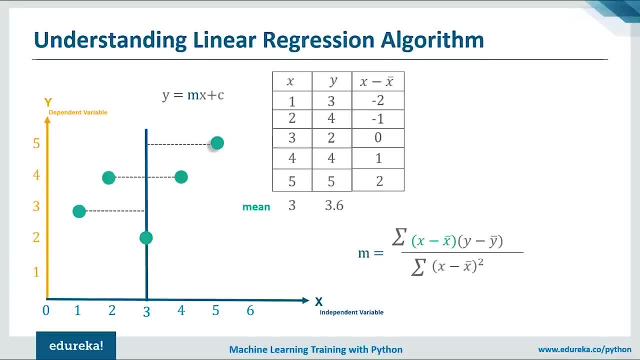 All right, so x minus x bar, It's nothing but the distance of all the point through the line y, equal 3. and what does this y minus y bar implies? it implies the distance Of all the point from the line x, equal 3.6. fine, 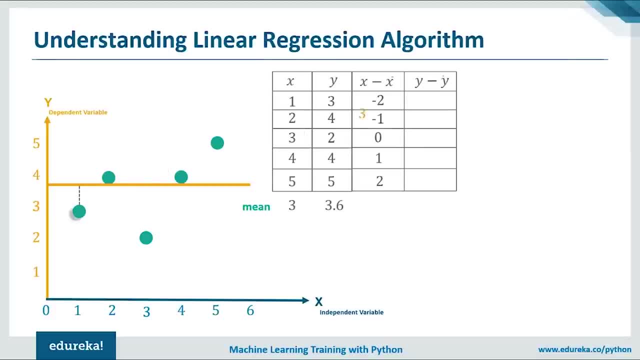 So let's calculate the value of y minus y bar. So, starting with y equal 3 minus value of y bar, that is 3.6.. So it is 3 minus 3.6.. How much minus of 0.6? next is 4 minus 3.6.. 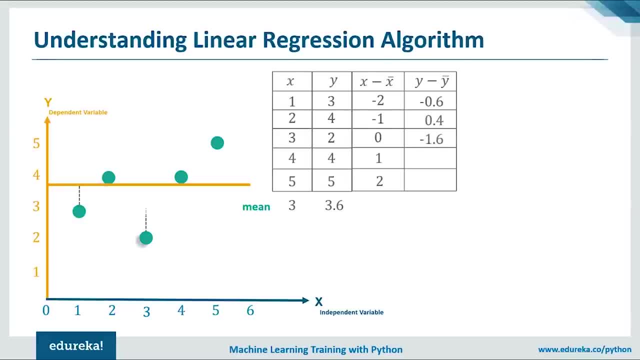 That is 0.4. next 2 minus 3.6.. That is minus of 1.6. next is 4 minus 3.6.. That is 0.4. again 5 minus 3.6.. That is 1.4.. 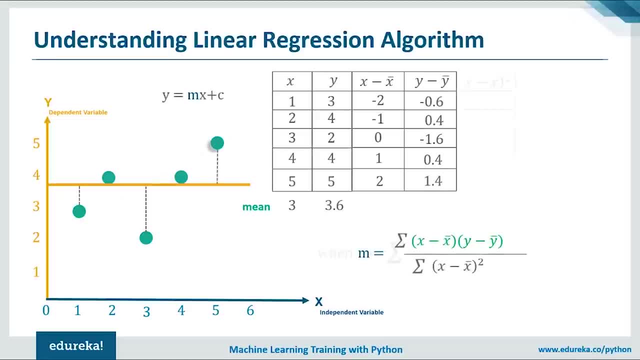 All right, So now we are done with y minus y, bar fine. Now next we'll calculate x minus x bar whole square. So let's calculate x minus x bar whole square, So it is minus 2 whole square, That is 4 minus 1 whole square. 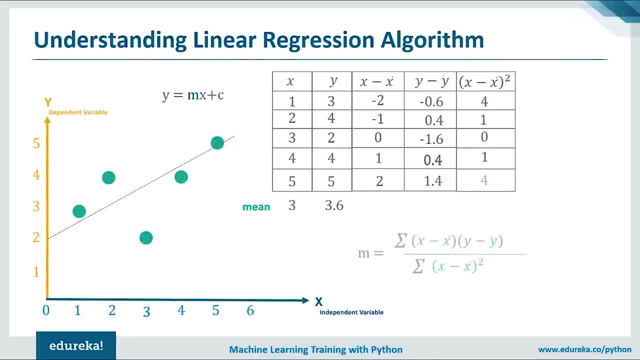 That is 1: 0 square 0, 1 square 1, 2 square 4. fine, So now in our table we have x minus x bar, y minus y bar and x minus x by whole square. Now what we need? we need the product of x minus x bar. 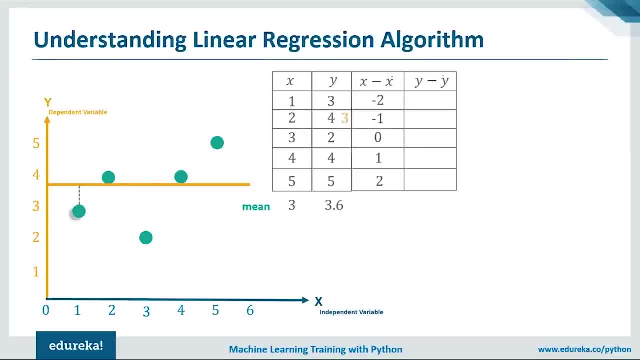 So let's calculate the value of Y minus Y bar. So, starting with Y equal 3 minus value of Y bar, that is 3.6.. So it is 3 minus 3.6.. How much minus of 0.6? next is 4 minus 3.6.. 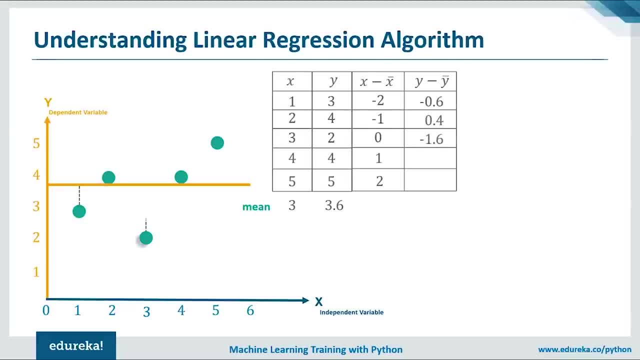 That is 0.4. next 2 minus 3.6.. That is minus of 1.6. next is 4 minus 3.6.. That is 0.4. again 5 minus 3.6.. That is 1.4.. 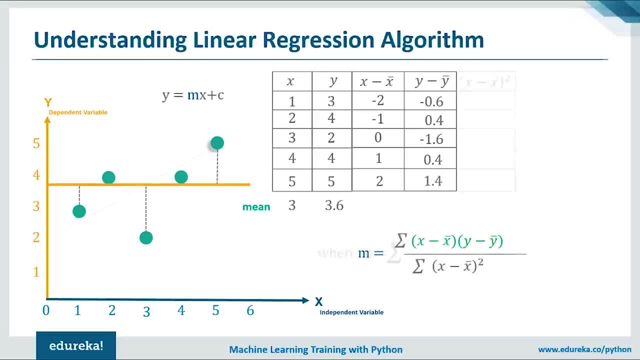 All right, So now we are done with Y minus Y. bar fine. Now next We'll calculate X minus X bar whole square. So let's calculate X minus X bar whole square, So it is minus two whole squared, That is four minus one whole squared. 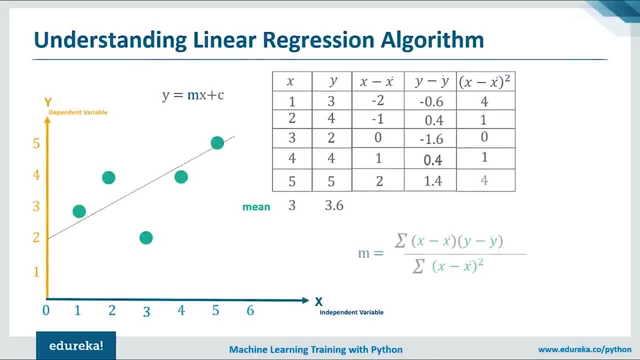 That is one zero square Zero. one square one, two square four. fine, So now in our table we have x minus X Bar, Y minus Y bar and X minus X bar whole square. Now what we need? We need the product of X minus X bar, x y Y bar. 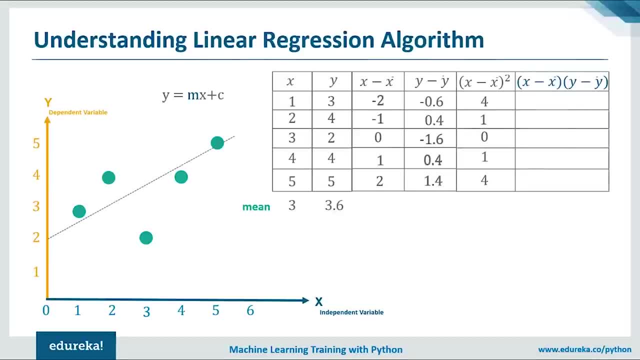 Alright, so let's see the product of X minus X bar, x. Y minus Y bar, that is minus of 2, multiplied by minus of 0.6, that is 1.2. minus of 1 multiplied by 0.4, that is minus of 0.4. 0 multiplied by minus of 1.6, that is 0. 1 multiplied by 0.4, that is 0.4. and next 2. 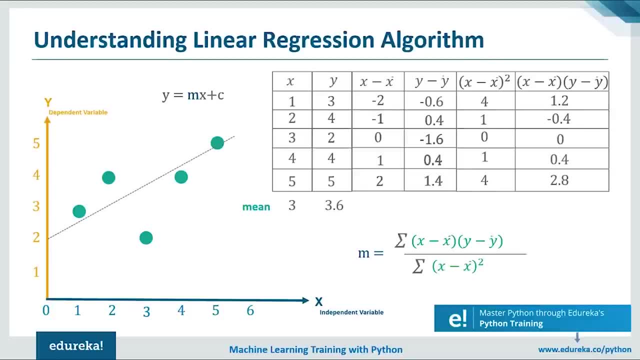 multiplied by 1.4, that is 2.8. all right, now, almost all the parts of our formula is done, so now what we need to do is get the summation of last two columns. all right, so the summation of x minus x bar whole square is 10, and the summation of x minus x bar multiplied by y minus y bar is 4. so 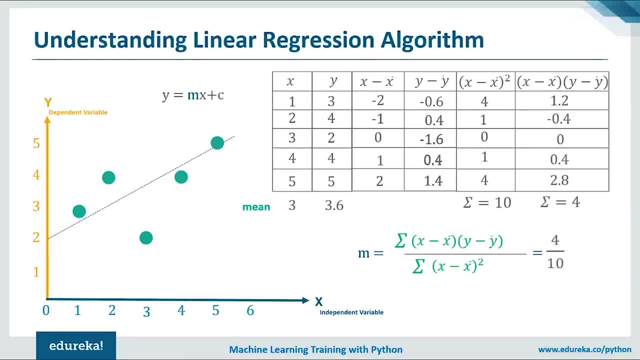 the value of m will be equal to 4 by 10. fine, so let's put this: value of m equals 0.4 in our line y, equal mx plus c. so let's fill all the points into the equation and find the value of c. so we: 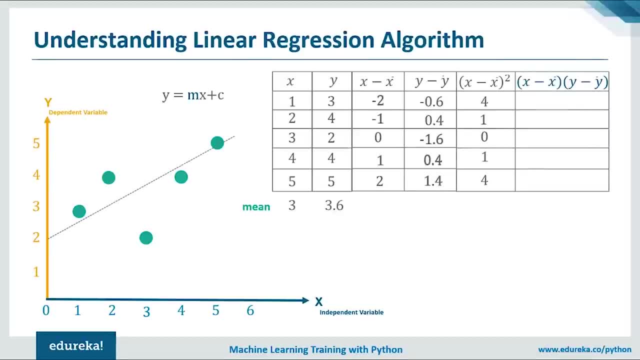 multiplication By y minus y bar. All right, so let's see the product of x minus x bar multiplied by y minus y bar, that is, minus of 2 multiplied by minus of 0.6.. That is, 1.2 minus of 1 multiplied by 0.4.. 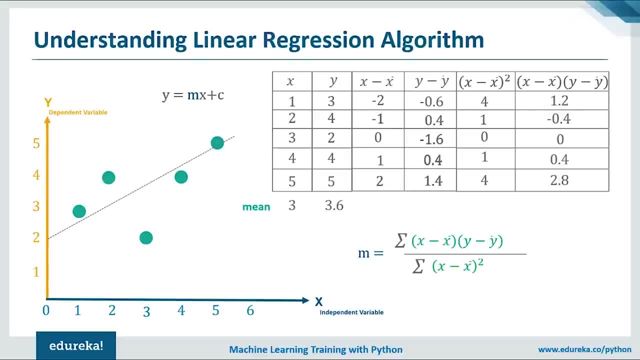 That is minus of 0.4. 0 multiplied by minus of 1.6.. That is 0, 1 multiplied by 0.4.. That is 0.4. and next 2 multiplied by 1.4.. That is 2.8.. 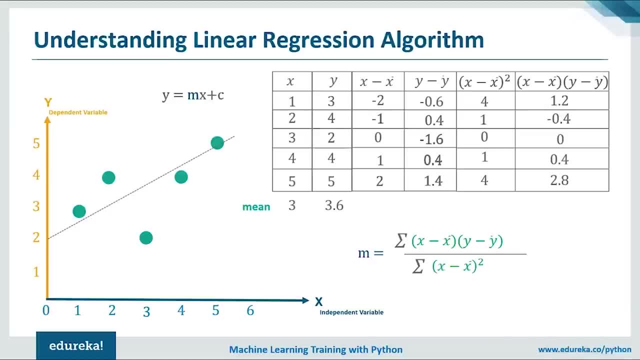 All right, now almost all the parts of our formula is done, So now what we need to do is get the summation of last two columns. All right, so the summation of x minus x bar whole square is 10, and the summation of x minus x bar multiplied by y minus y. 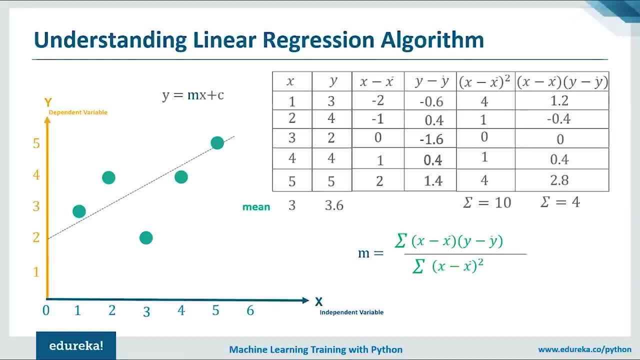 bar is 4.. So the value of M will be equal to 4 by 10. fine, So let's put this: value of M equals 0.4 in our line, y equal MX plus C. So let's fill all the points into the equation and find the. 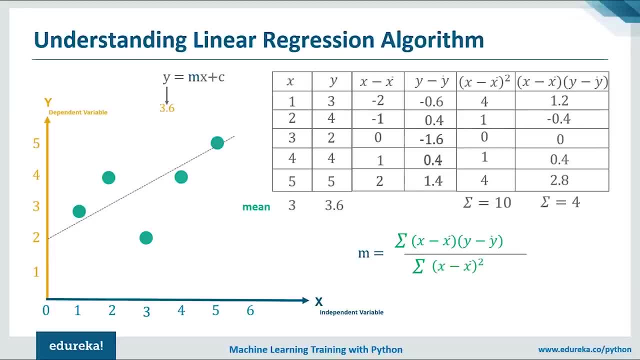 value of C. So we have y as 0.6.. Remember the mean y M as 0.4, which we calculated just now: X as the mean value of X, that is 3, and we have the equation as: 3.6 equals 0.4 multiplied by 3. 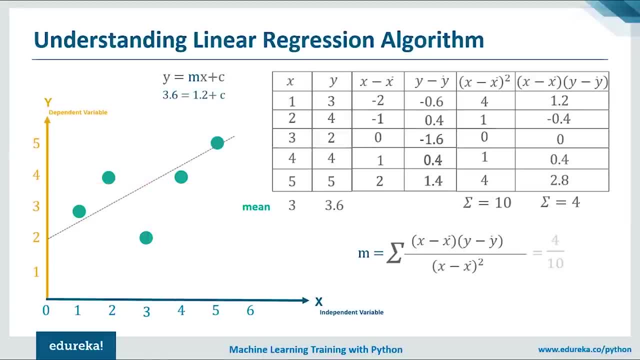 plus C. All right, that is 3.6 equals 1.2 plus C. So what is the value of C? that is 3.6 minus 1.2, that is 2.4.. All right, So what we had? we had M equals 0.4 C as 2.4.. 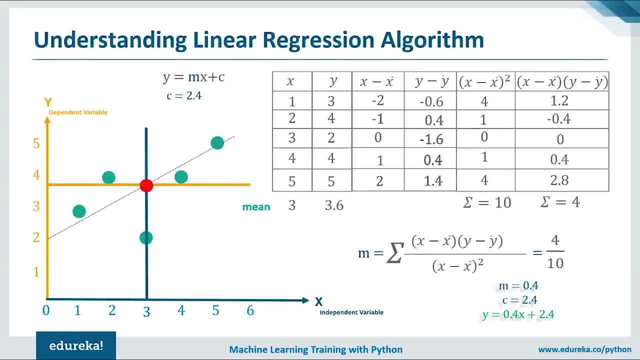 And then, finally, when we calculate the equation of regression line, what we get is y equal 0.4 times of X plus 2.4.. So this is the regression line. All right, So there's how you are plotting your points. 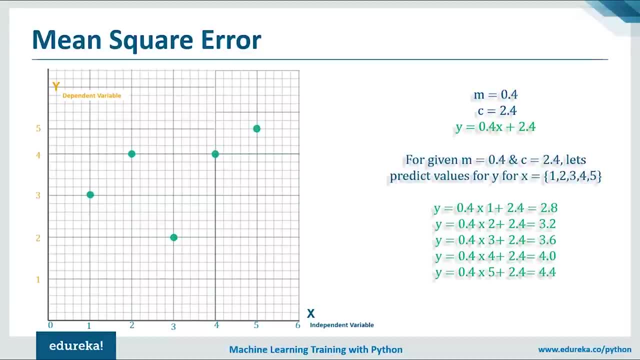 This is your actual point. All right now, for given M equals 0.4 and C equal 2.4.. Let's predict the value of y for x equal 1, 2, 3, 4 and 5.. So when x equals 1, the predicted value of y will be 0.4 multiplied. 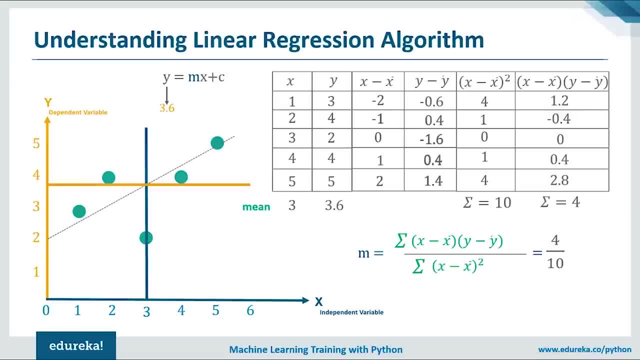 have y as 3.6. you remember the mean y, m as 0.4, which we calculated just now. x as the mean value of x, that is 3, and we have the equation as: 3.6 equals 0.4 multiplied by 3 plus c. all right, that is 3.6. 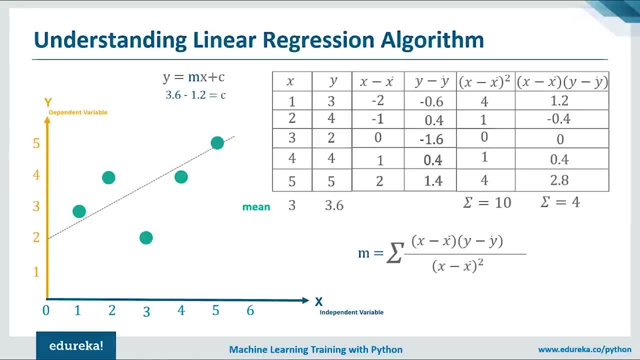 equal 1.2 plus c. so what is the value of c? that is 3.6 minus 1.2, that is 2.4. all right, so what we had? we had m equals 0.4, c as 2.4. and then, finally, when 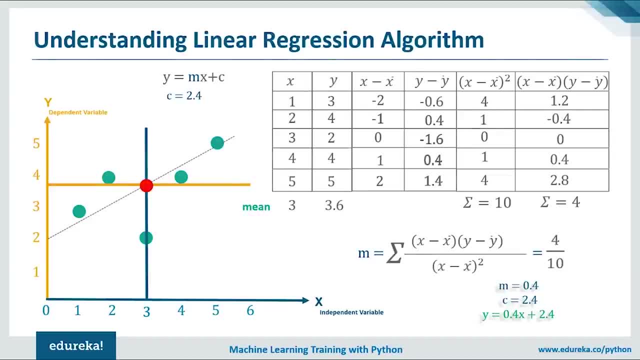 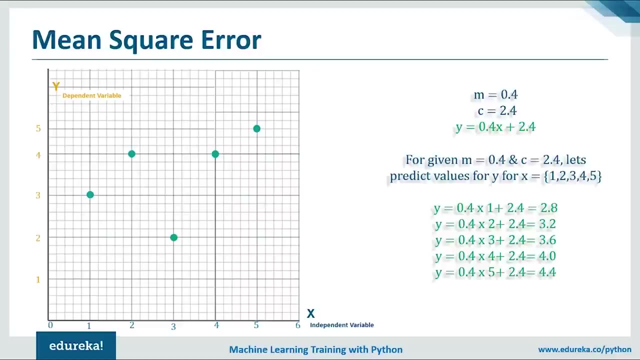 we calculate the equation of regression line, what we get is y equal 0.4 times of x plus 2.4. so this is the regression line. all right, so there's how you are plotting your points. this is your actual point. all right now, for given m equals 0.4 and c equal 2.4, let's predict the value of y. 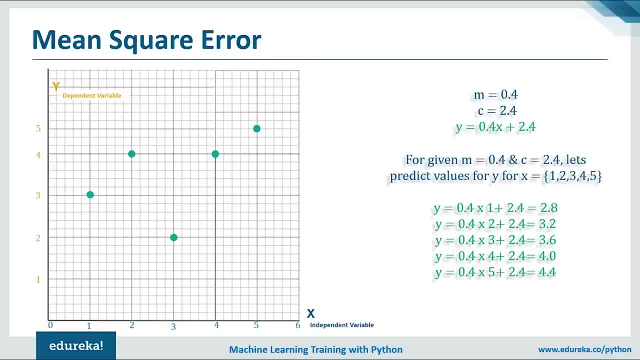 for x equal 1, 2, 3, 4 and 5.. so, when x equal 1, the predicted value of y will be 0.4 multiplied by 1 plus 2.4, that is, 2.8. similarly, when x equal 2, predicted value of y will be 0.4 multiplied by 2 plus 2.4. 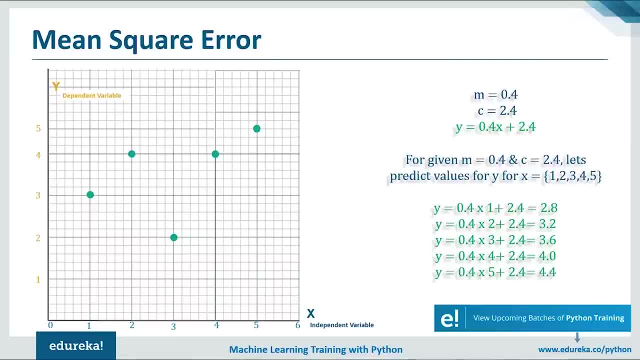 that equals to 3.2. similarly, x equal 3, y will be 3.6. x equal 4, y will be 4.0. x equal 5, y will be 4.4. so let's plot them on the graph and the line passing through all these predicting point and 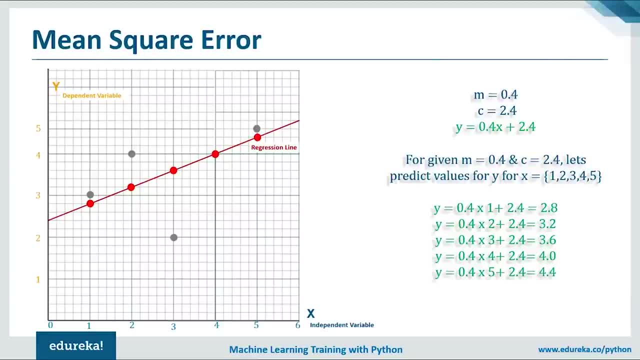 cutting y axis at 2.4 is the line of regression. now your task is to calculate the distance between the actual and the predicted value, and your job is to reduce the distance. all right, or in other words, you have to reduce the error between the actual and the. 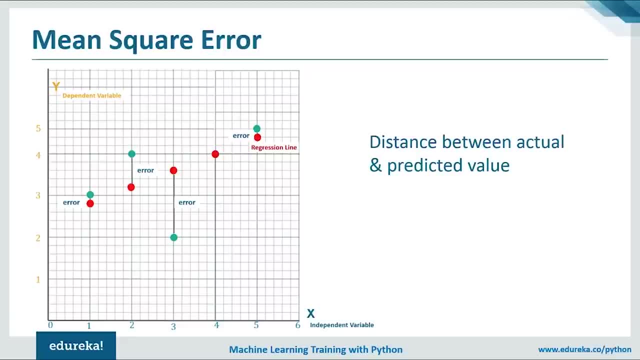 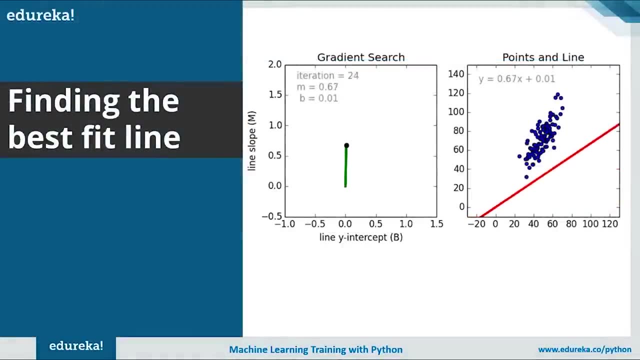 predicted value. the line with the least error will be the line of linear regression or regression line, and it will also be the best fit line. all right, so this is how things work in computer. so what it do? it performs n number of iteration for different values of m. for different values of m, it will 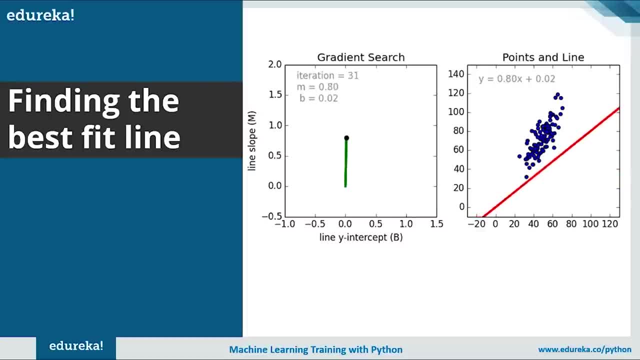 calculate the equation of line where y equal m plus c, right. so as the value of m changes, the line is changing. so iteration will start from one, all right, and it will perform n number of iteration. so after every iteration, what it will do? it will calculate the predicted value according to the line and compare the distance of actual value to 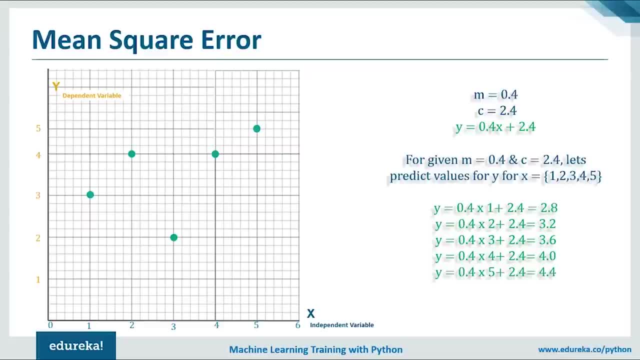 by 1 plus 2.4.. That is 2.8. similarly, when x equal 2, predicted value of y will be 0.4 multiplied by 2 plus 2.4, that equals to 3.2.. Similarly, x equal 3, y will be 3.6. x equal 4, y will be 4.0. x. 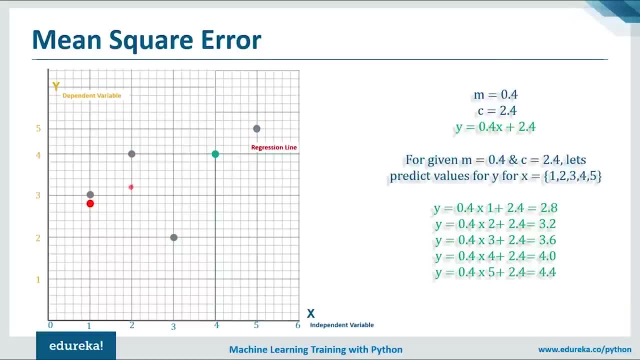 equal 5, y will be 4.4.. So let's plot them on the graph, and the line passing through all these predicting point and cutting y-axis at 2.4 is the line of regression. Now your task is to calculate the distance between the actual 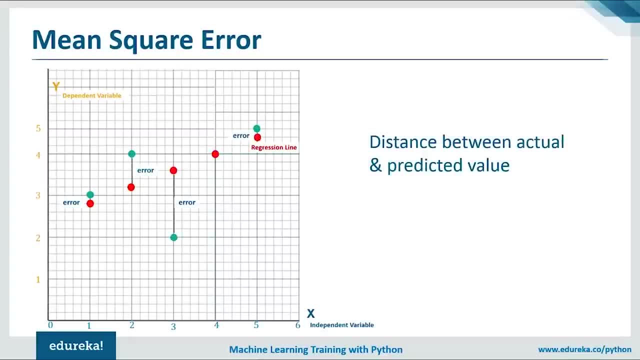 and the predicted value, and your job is to reduce the distance LA, or in other words, you have to reduce the error between the actual and the predicted value. the line with the least error will be the line of linear regression or regression line, and it will also be the best-fit line. 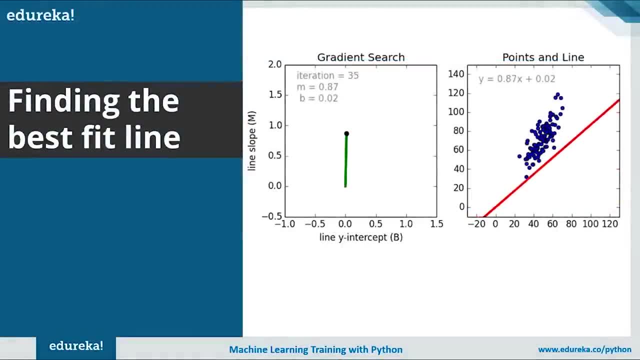 All right. So this is how things work in computer. So what it do? it performs n number of iteration for different values of M. for different values of M, It will calculate the equation of line. We have y equal MX plus C, right? So as the value of M changes, the line is changing. 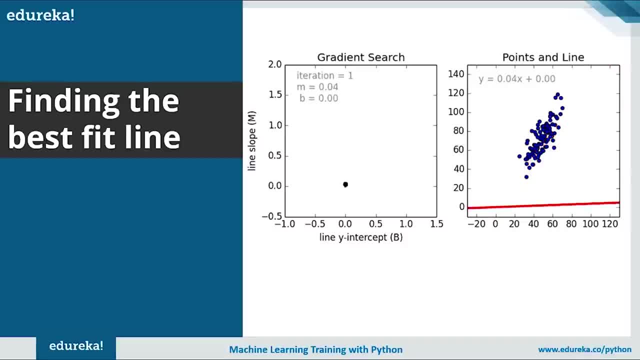 So iteration will start from one, all right, and it will perform n number of iteration. So after every iteration, what it will do? it will calculate the predicted value according to the line and compare the distance of actual value to the predicted value and the value of M, for which the distance 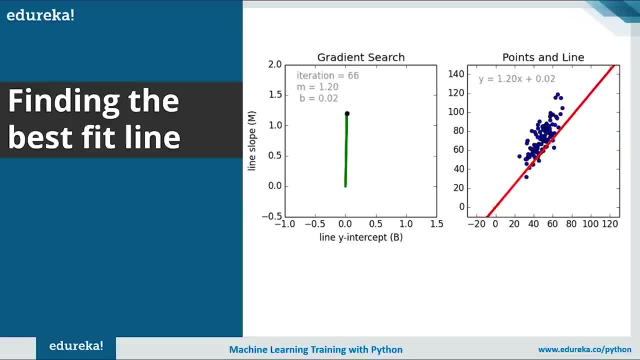 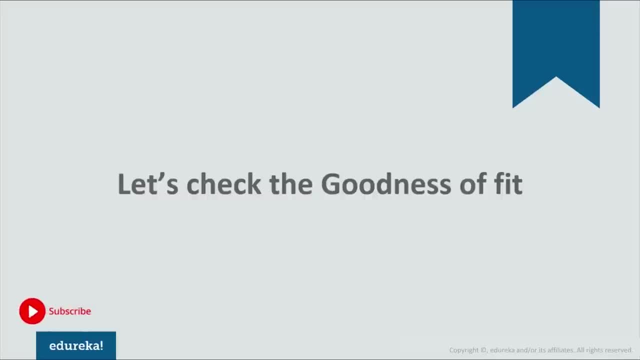 between the actual and the predicted value is minimum will be selected as the best-fit line. All right, Now that we have calculated the best-fit line, now it's time to check the goodness of it, or to check how good a model is performing. 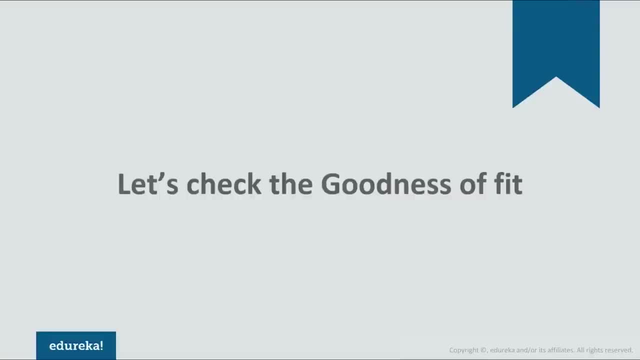 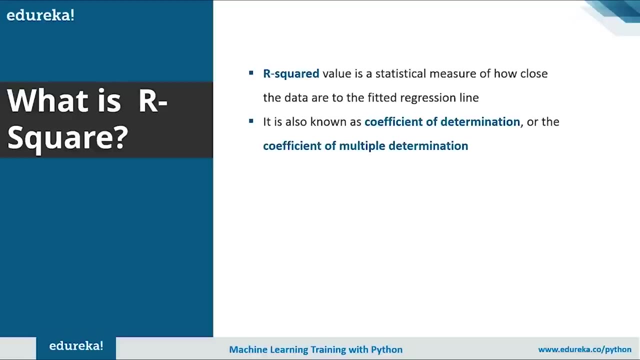 So, in order to do that, we have a method called R square method. So what is this R square? Well, R squared value is a statistical measure of how close the data are to the fitted regression line. in general, It is considered that a higher squared value model 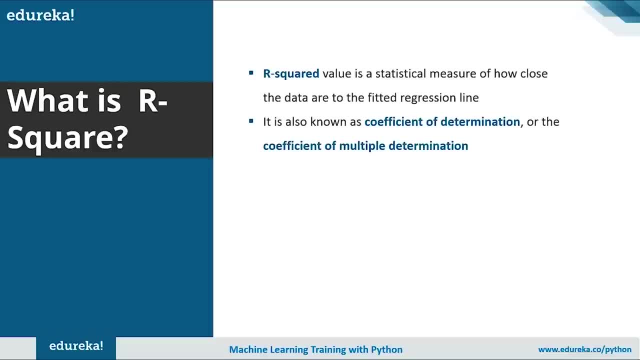 is a good model, but you can also have a lower squared value for a good model as well, or a higher squared value for a model that does not fit at all. All right, it is also known as coefficient of determination or the coefficient of multiple determination. 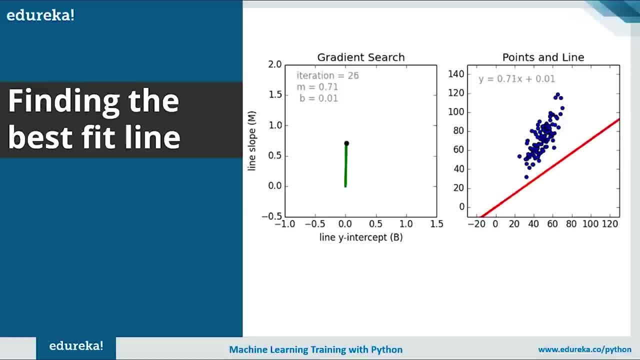 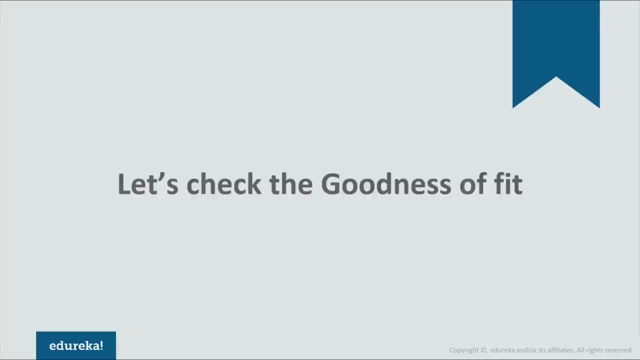 the predicted value and the value of m, for which the distance between the actual and the predicted value is minimum, will be selected as the best fit line. all right, now that we have calculated the best fit line, now it's time to check the goodness of fit, or to check how good a model is performing. so, in order to do that, 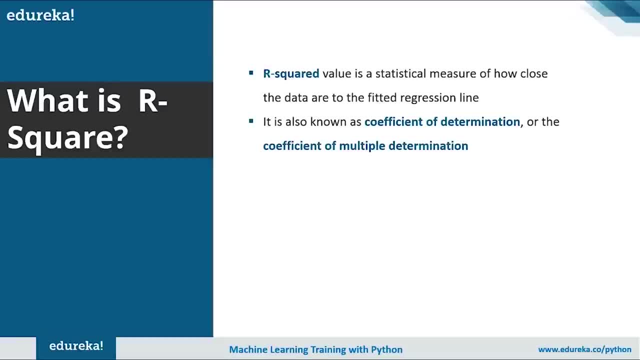 we have a method called r square method. so what is this r square? well, r squared value is a statistical measure of how close the data are to the fitted regression line. in general, it is considered that a higher squared value model is a good model, but you can also have a lower squared value for a good. 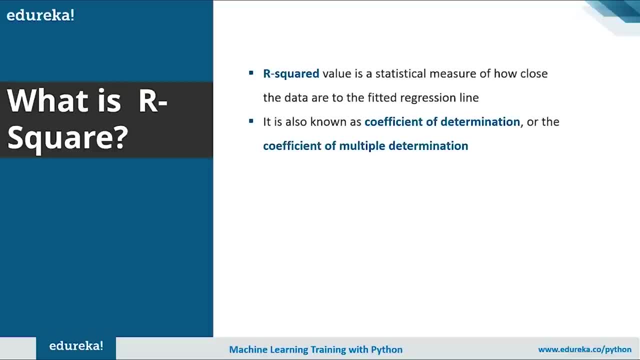 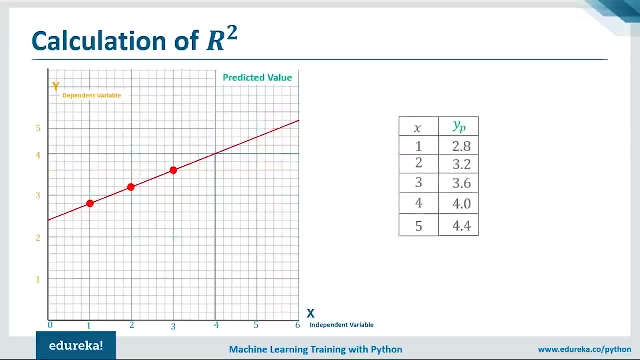 model as well, or a higher squared value for a model that does not fit at all. all right, it is also known as coefficient of determination or the coefficient of multiple determination. let's move on and see how r square is calculated. so these are our actual values, plotted on the graph. we had calculated the predicted values of y as 2.8, 3.2. 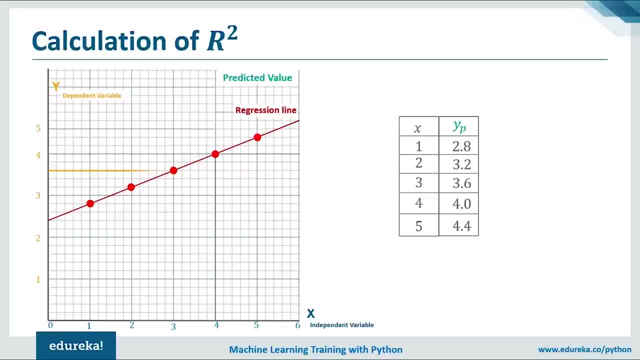 3.6, 4.0, 4.4. remember when we calculated the predicted values of y for the equation: y predicted equals 0.4 times of x plus 2.4. for every x equal 1, 2, 3, 4 and 5. from there we got the predicted. 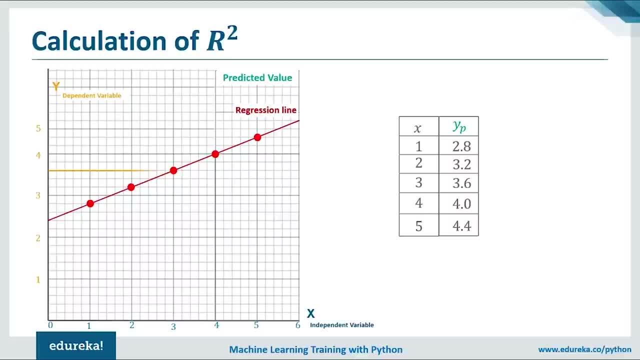 values of y. all right, so let's plot it on the graph. so these are a point and the line passing through these points are nothing but the regression line. all right, now what you need to do is you have to check and compare the distance of actual minus mean. 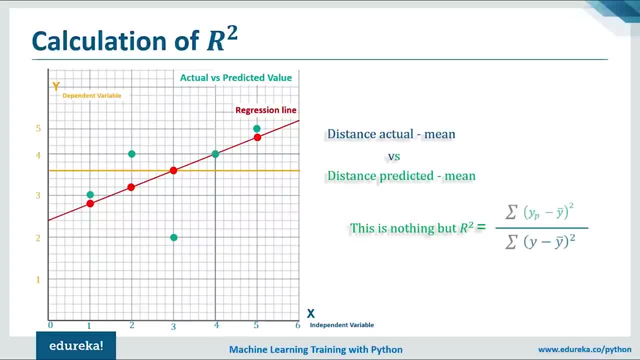 versus the distance of predicted minus mean. all right. so basically what you're doing, you're calculating the distance of actual value to the mean to distance of predicted value to the mean. all right. so there's nothing but r? square and mathematically you can represent r? square as: 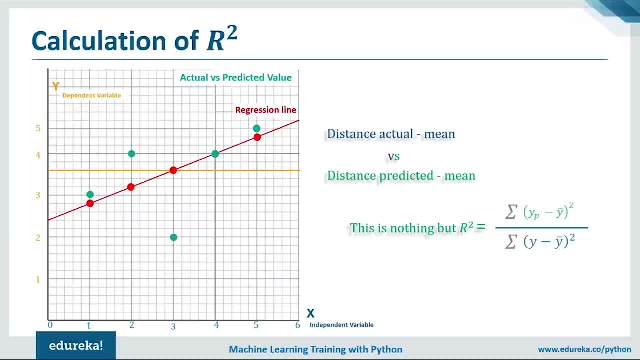 summation of y predicted values minus y bar: whole square. divided by summation of y minus y bar: whole square, where y is the actual value, yp is the predicted value and y bar is the mean value of y, that is nothing but 3.6. so remember, this is our. 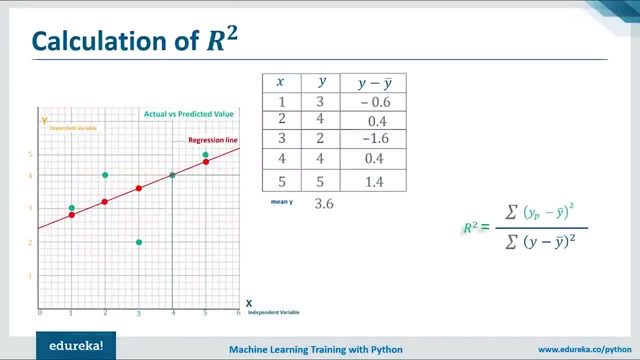 formula. so next what we'll do. we'll calculate y minus y bar, so we have y as 3, y bar as 3.6, so we'll calculate it as 3 minus 3.6, that is nothing but minus of 0.6. similarly, for y equal. 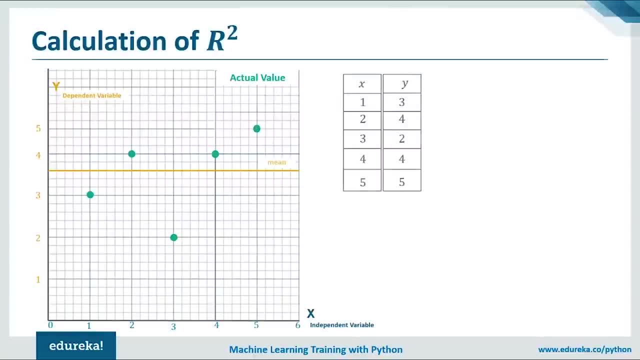 Let's move on and see how R square is calculated. So these are our actual values plotted on the graph. We had calculated the predicted values of Y as 2.8, 3.2,, 3.6,, 4.0, 4.4.. 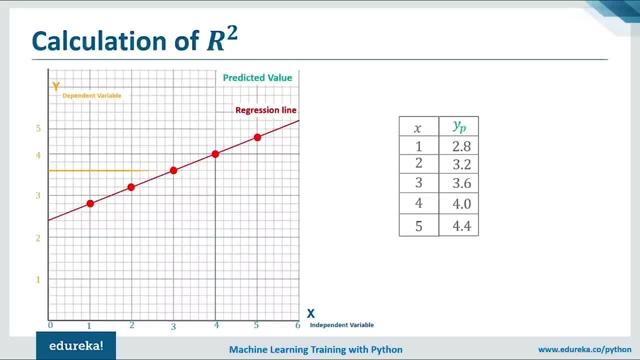 Remember when we calculated the predicted values of Y for the equation Y predicted equals 0.4 times of X plus 2.4. for every X equal 1, 2, 3, 4 and 5. from there We got the predicted values of Y. 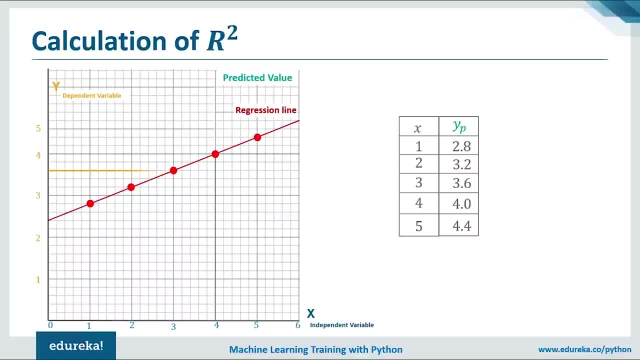 All right, So let's plot it on the graph. So these are a point and the line passing through these points are nothing but the regression line. All right, Now what you need to do is you have to check and compare the distance of actual minus mean. 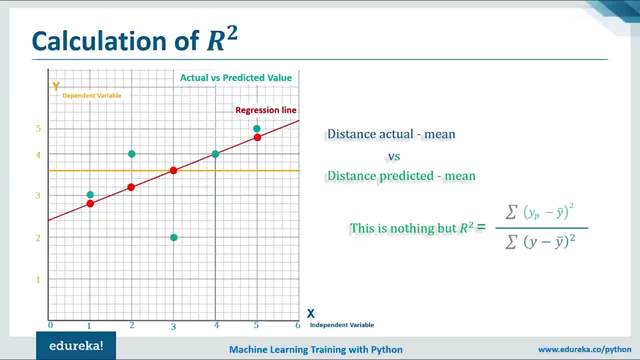 versus the distance of predicted minus mean. All right. So basically what you're doing, you're calculating the distance of actual value to the mean to distance of predicted value to the mean. All right, So there's nothing but R square in. mathematically, you can represent R square. 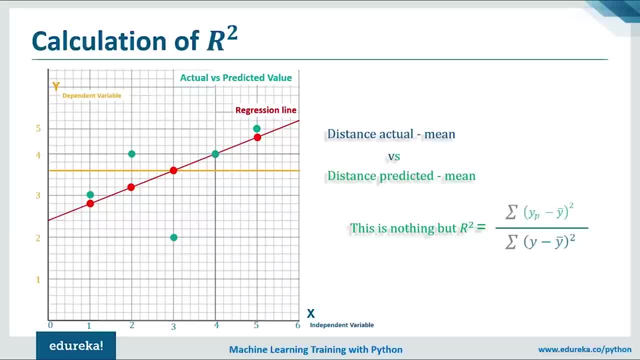 as summation of Y predicted values minus Y bar: whole square divided by summation of Y minus Y bar: whole square where Y is the actual value, YP is the predicted value and Y bar is the mean value of Y, that is nothing but 3.6.. 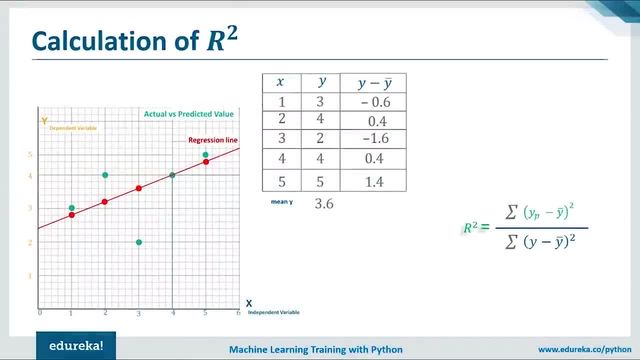 So remember, this is our formula. So next, what we'll do will calculate Y minus Y bar. So we have Y as 3, Y bar as 3.6.. So we'll calculate it as 3 minus 3.6.. That is nothing but minus of 0.6.. 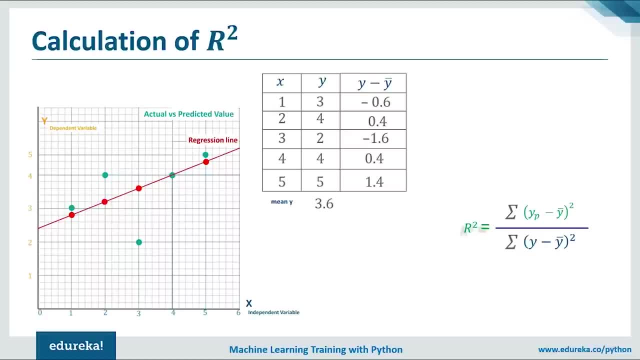 Similarly for Y equal 4 and Y bar equal 3.6.. We have Y minus Y bar as 0.4, then 2 minus 3.6.. It is 1.6, 4 minus 3.6, again 0.4, and 5 minus 3.6.. 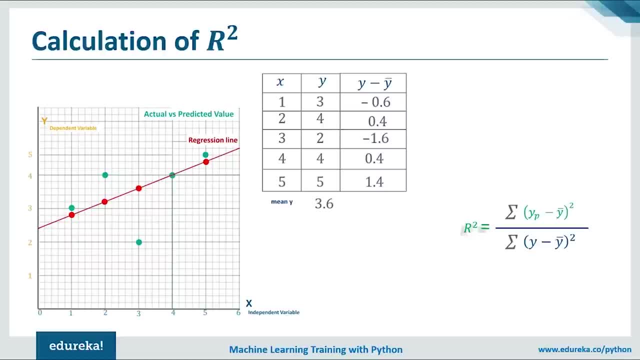 It is 1.4.. So we got the value of Y minus Y bar. Now what we have to do? we have to take it square. So we have minus of 0.6 square as 0.36. 0.4 square as 0.16 minus. 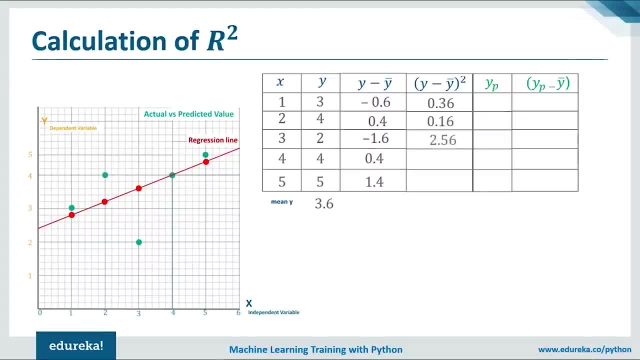 of 1.6 square as 2.56, 0.4 square as 0.16 and 1.4 square as 1.96.. Now, as a part of formula, what we need? we need our YP minus Y bar value. 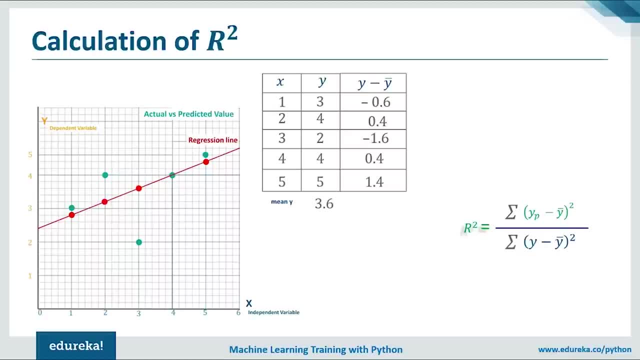 4 and y bar equal 3.6. we have y minus y bar as 0.4. then 2 minus 3.6, it is 1.6, 4 minus 3.6, again 0.4, and 5 minus 3.6, it is 1.4. so we got. 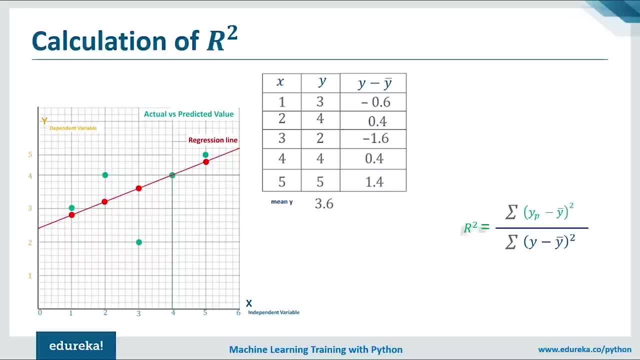 the value of y minus y bar. now, what we have to do, we have to take it square. so we have minus of 0.6 square as 0.36, 0.4 square as 0.16, minus of 1.6 square as 2.56, 0.4 square as 0.16, and 1.4. 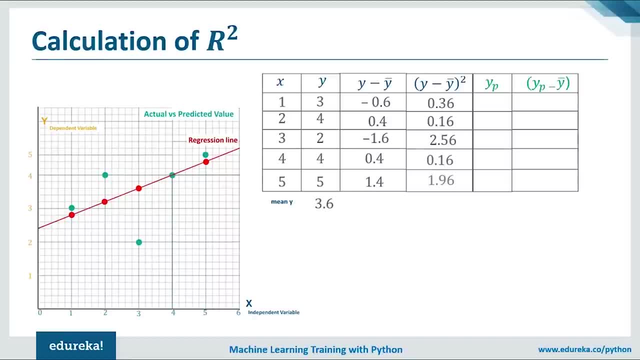 square as 1.96. now, as a part of formula, what we need? we need our yp minus y bar value. so these are yp values and we have to subtract it from the mean of y. so 2.8 minus 3.6, that is, minus 0.8. 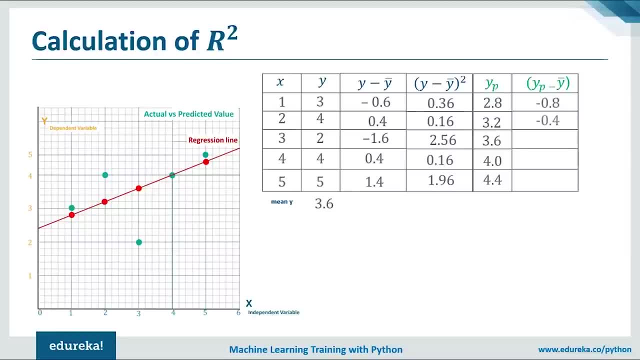 similarly, we'll get 3.2 minus 3.6, that is 0.4, and 3.6 minus 3.6, that is 0. 4.0 minus 3.6, that is 0.4, then 4.4 minus 3.6, that is 0.8. so we calculated the value of yp. 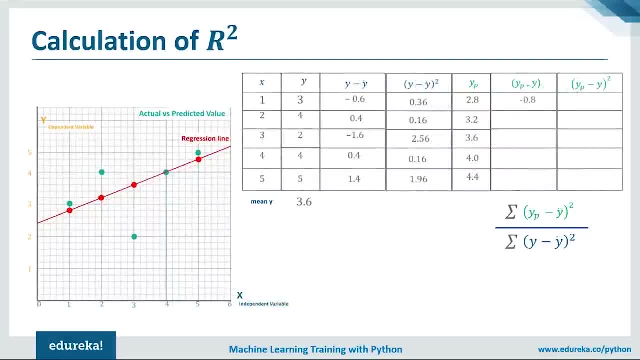 minus y bar. now it's our turn to calculate the value of yp minus y bar whole square. next we have minus of 0.8 square as 0.64. minus of 0.4 square as 0.16. 0 square 0 0.4 square as again 0.16. 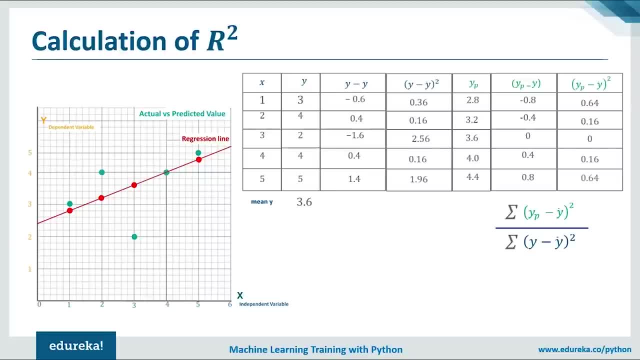 and 0.8 square as 0.64. all right, now, as a part of formula, what it suggests? it suggests me to take the summation of yp minus y bar whole square and summation of y minus y bar whole square. all right, let's see. so, on summating y minus y bar whole square, what you get is 5.2 and summation of. 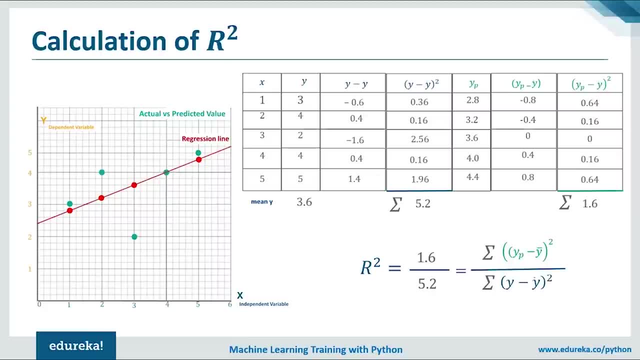 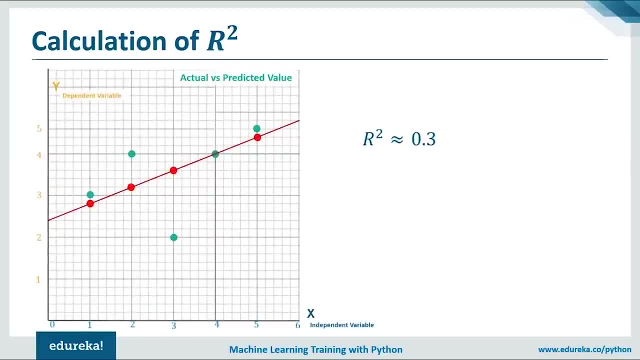 yp minus y, bar whole square, you get 1.6. so the value of r square can be calculated as 1.6 upon 5.2. fine, so the result which you will get is approximately equal to 0.3. well, this is not a. 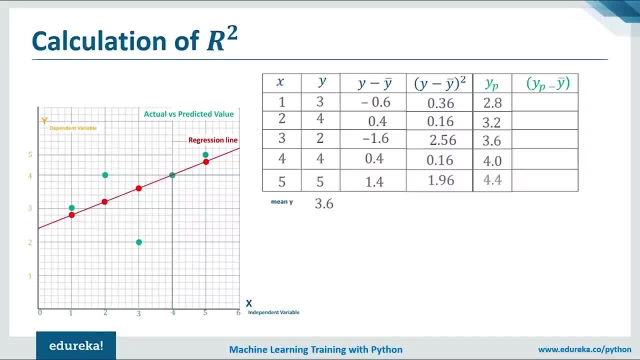 So these are YP values and we have to subtract it from the mean of Y, so 2.8 minus 3.6, that is minus 0.8.. Similarly, we'll get 3.2 minus 3.6.. That is 0.4 and 3.6 minus 3.6.. 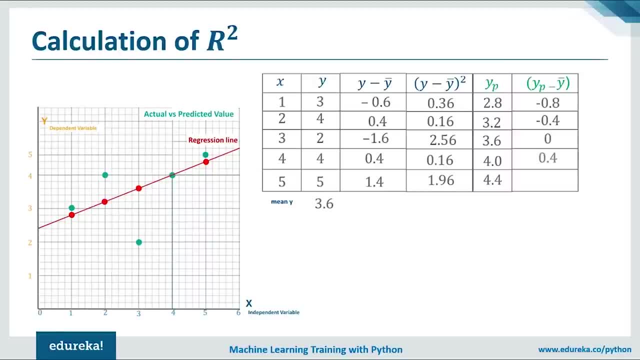 That is 0, 4.0 minus 3.6.. That is 0.4. then 4.4 minus 3.6.. That is 0.8.. So we calculated the value of YP minus Y bar. Now it's our turn to calculate the value of YP minus Y bar. 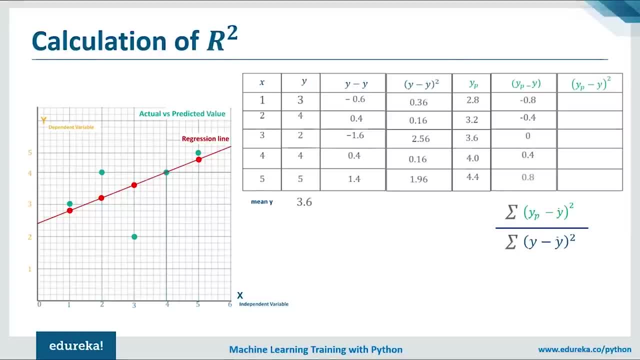 whole square. Next, we have minus of 0.8 square as 0.64. minus of 0.4 square as 0.16. 0 square 0, 0.4 square, as again 0.16 and 0.8 square. 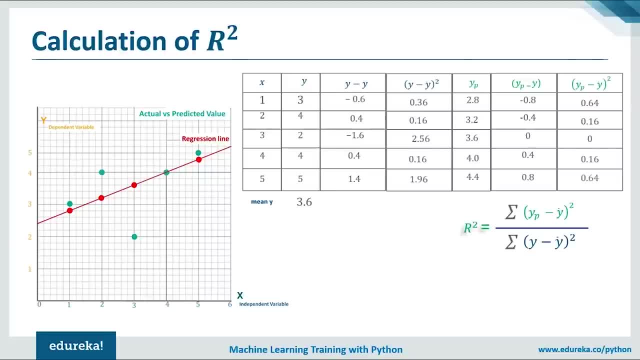 as 0.64.. All right now, as a part of formula, what it suggests. it suggests me to take the summation of YP minus Y bar whole square and summation of Y minus Y bar whole square. All right, let's see. so, on submitting Y minus Y bar whole, 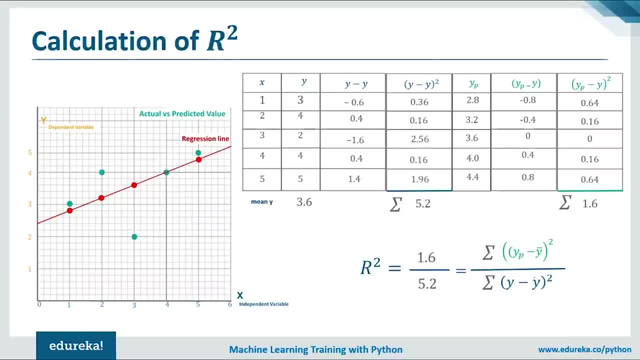 square, what you get is 5.2, and summation of YP minus Y bar whole square, you get 1.6.. So the value of R square can be calculated as 1.6 upon 5.2. fine, So the result which you will get is approximately equal to 0.3.. 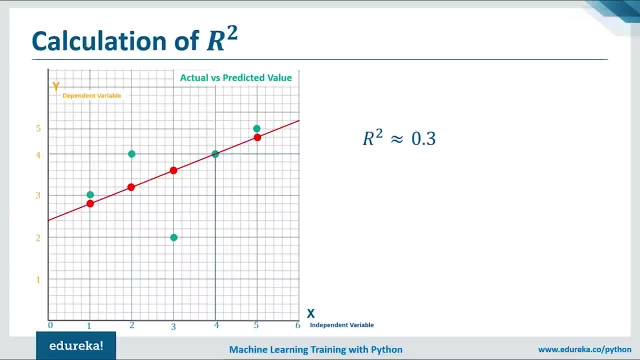 Well, this is not a good fit. All right, so it suggests that the data points are far away from the regression line. All right, So this is how you do it. This is how your graph will look like when R square is 0.3. 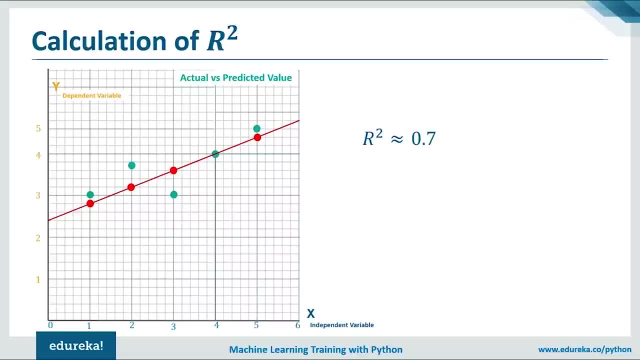 when you increase the value of R square to 0.7.. So you'll see that the actual value would lie closer to the regression line when it reaches to 0.9.. It comes more close, and when the value approximately equals to 1, then the actual values lies on the regression line itself. 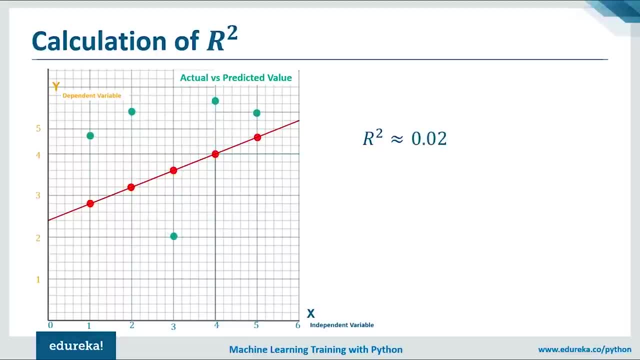 For example, in this case, if you get a very low value of R square, suppose 0.02.. So in that case what you'll see? that the actual values are very far away from The regression line, or you can say that there are too many. 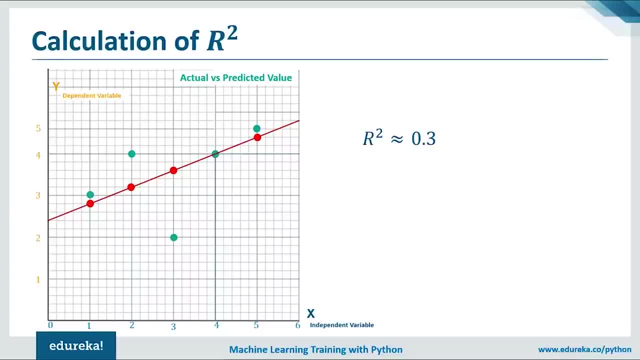 good fit. all right, so it suggests that the data points are far away from the regression line. all right, so this is how your graph will look like when r square is 0.3. when you increase the value of r square to 0.7, so you'll see that the actual value would 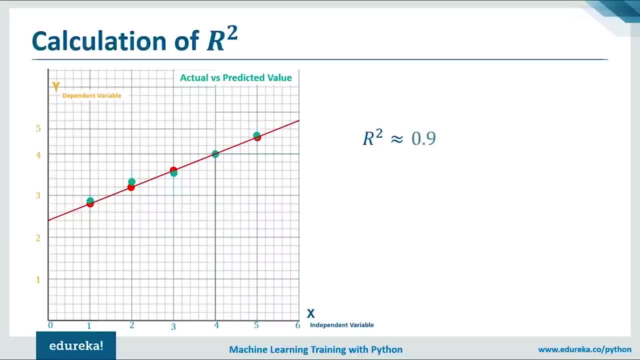 lie closer to the regression line. when it reaches to 0.9, it comes more close, and when the value approximately equals to 1, then the actual values lies on the regression line itself. for example, in this case, if you get a very low value of r square, suppose 0.02. so in that case what you'll see? that 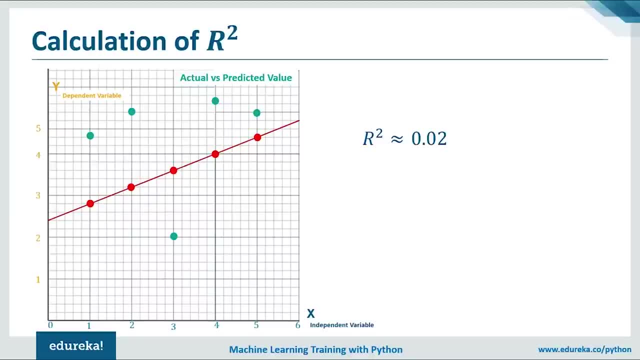 the actual values are very far away from the regression line, or you can say that there are many outliers in your data. you cannot forecast anything from the data, all right, so this was all about the calculation of r square. now you might get a question like: are low values of r square? 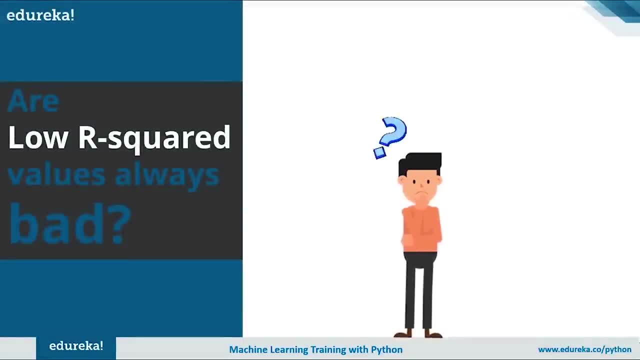 always bad. well, in some field, it is entirely expected that our r square value will be low. for example, any field that attempts to predict human behavior, such as psychology, typically has r squared values lower than around 50, through which you can conclude that humans are simply harder to predict than the physical process. 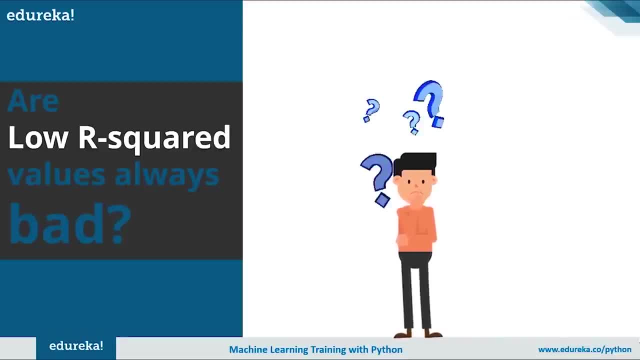 furthermore, if your r squared value is low but you have statistically significant predicators, then you can still draw important conclusion about how changes in the predicator values are associated with the changes in the response value. regardless of the r squared, the significant coefficient still represent the mean change in the response for one unit of change in the predicator. 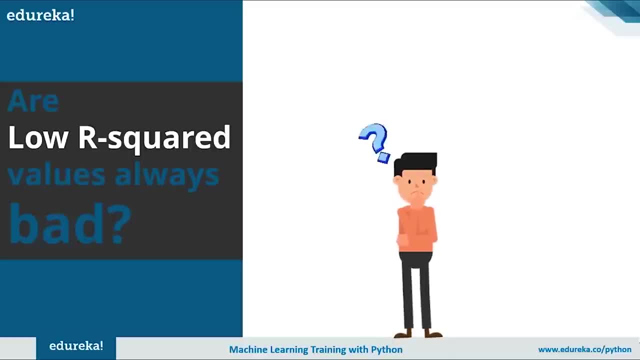 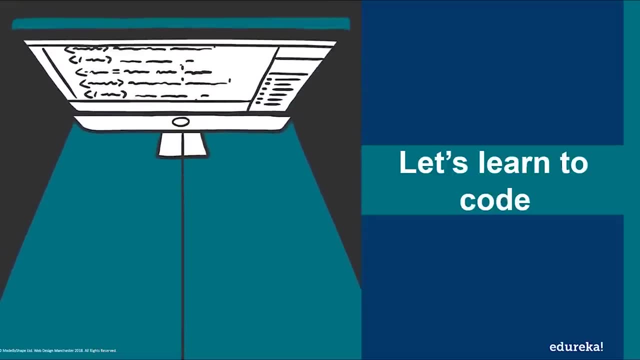 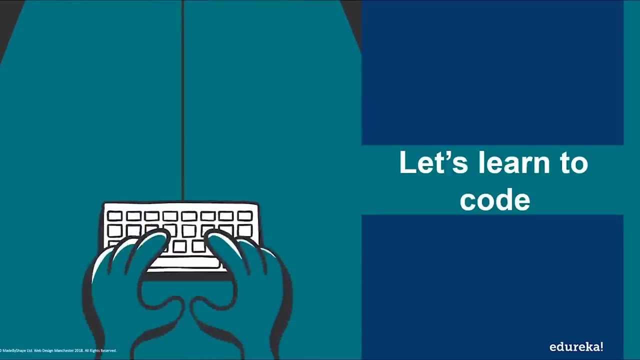 while holding other predicators in the model constant. obviously, this type of information can be extremely valuable. all right, all right. so this was all about the theoretical concept. now let's move on to the coding part and understand the code in depth. so for implementing linear regression using python, i'll be using anaconda with jupiter notebook. 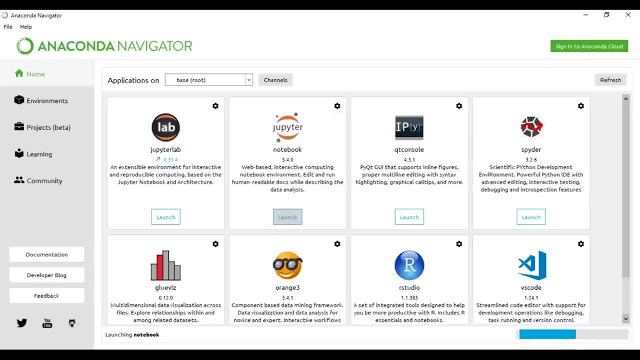 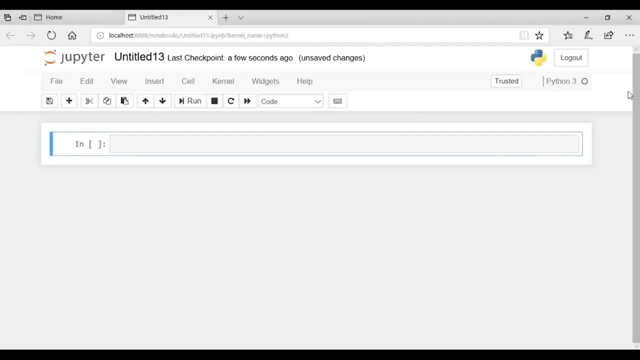 installed on it. so, all right, this is our jupiter notebook and we are using python 3.0 on it. all right, so we are going to use a data set consisting of head size and human brain of different people. all right, so let's import our data set, percent matplotlib- in line. we are importing numpy as np. 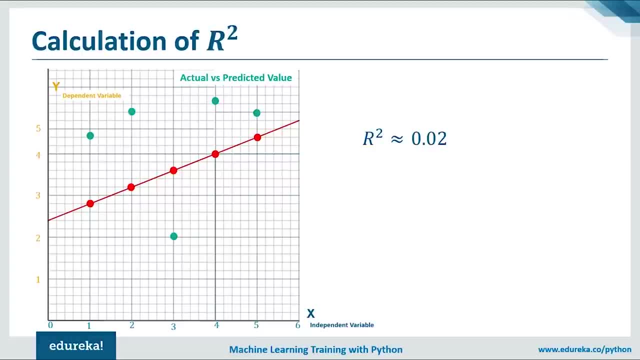 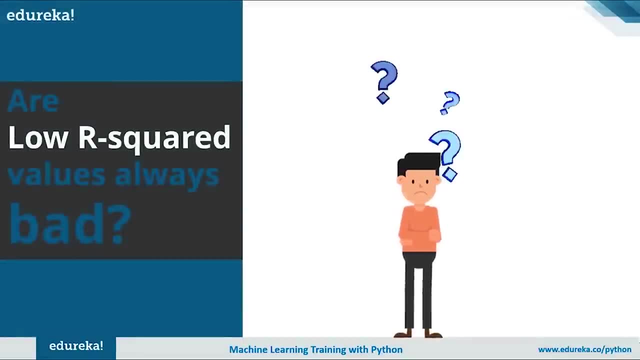 outliers in your data. You cannot focus anything from the data. All right, so this was all about the calculation of R square. Now you might get a question: like our low values of R square always bad? Well, in some field it is entirely expected that our R. 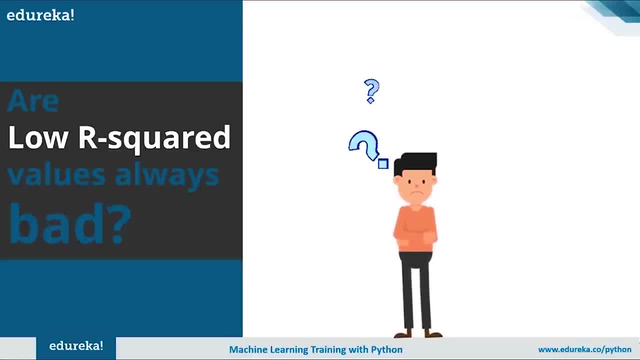 square value will be low. For example, any field that attempts to predict human behavior, such as psychology, typically has R squared values lower than around 50%, through which you can conclude that humans Are simply harder to predict than the physical process. Furthermore, if your R squared value is low, but you have 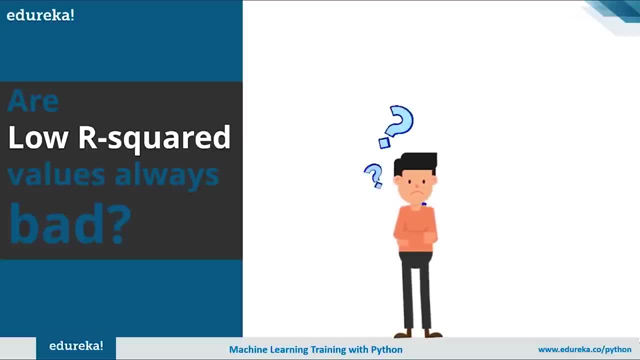 statistically significant predicators, then you can still draw important conclusion about how changes in the predicator values are associated with the changes in the response value. regardless of the R squared, the significant coefficient still represent the mean change in the response for one unit of change in the predicator, while holding other predicators in. 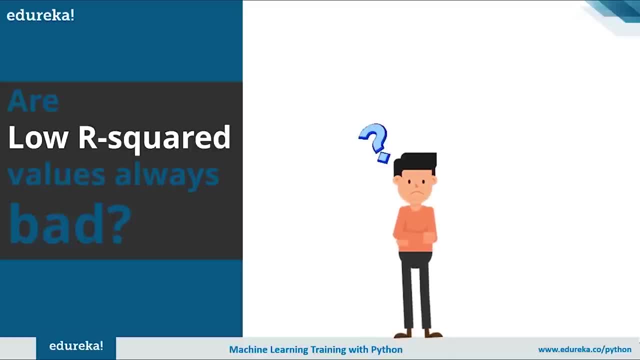 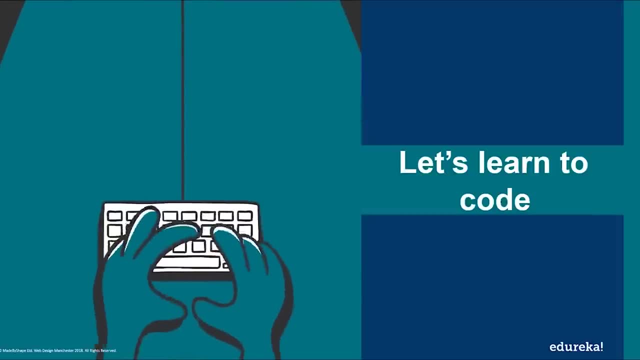 the model constant. obviously, this type of information can be extremely valuable. All right, All right. So this was all about the theoretical concept. Now let's move on to the coding part and understand the code in depth. So, for implementing linear regression using python, I'll 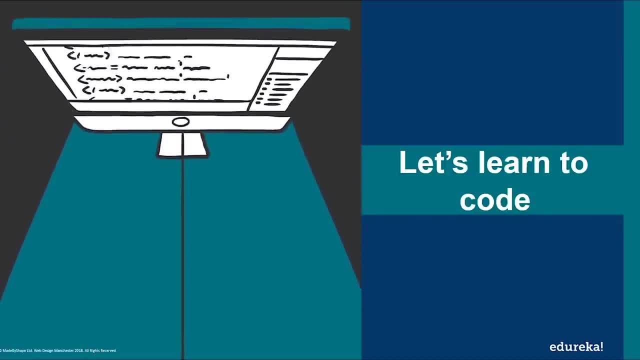 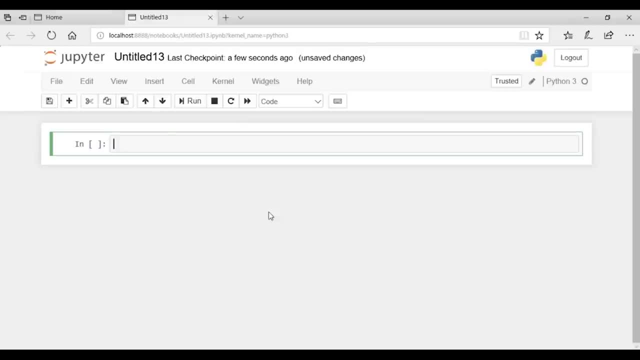 be using anaconda with Jupiter notebook installed on it. So, all right, this is our Jupiter notebook and we are using python 3.0 on it. All right, So we are going to use a data set consisting of head size and human brain of different people. 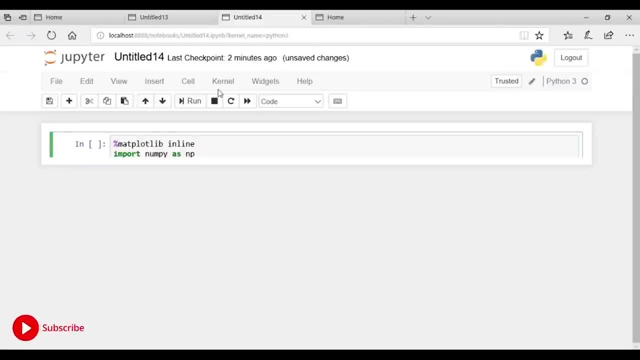 All right. So let's import our data set percent matplotlib. In line. We are importing numpy as NP, pandas as PD and matplotlib, and from matplotlib We are importing pi plot of that as PLT. All right, Next we'll import our data head brain dot CSV and store it. 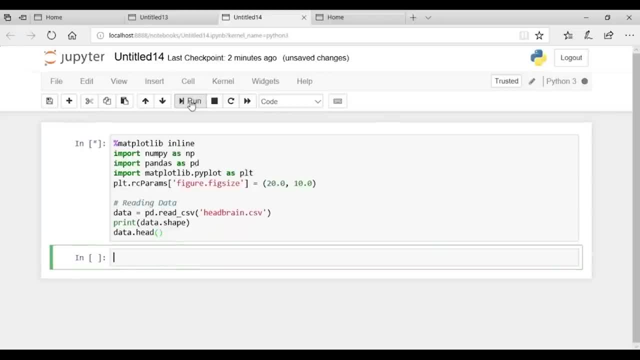 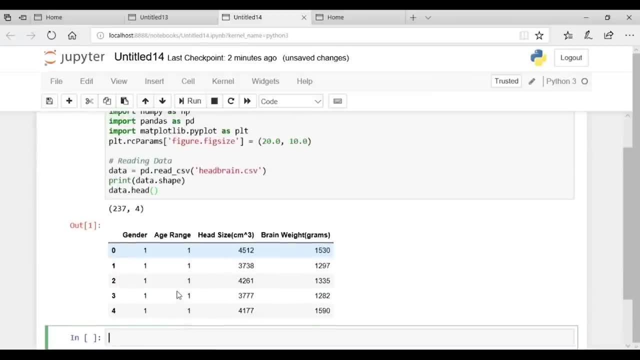 in the data variable. Let's execute the run button and see the output. So this asterisk symbol. it symbolizes that it's still executing. So there's a output. our data set consists of 237 rows and four columns. We have columns as gender, age range, head size. 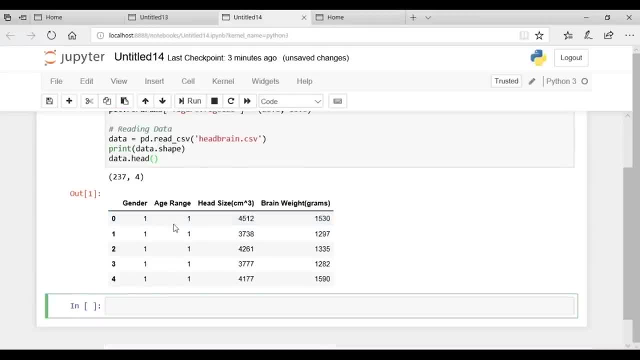 In centimeter Q and brain weights in gram fine. So there's a sample data set. This is how it looks. it consists of all these data set. So now that we have imported our data. So, as you can see, there are 237 values in the training set. 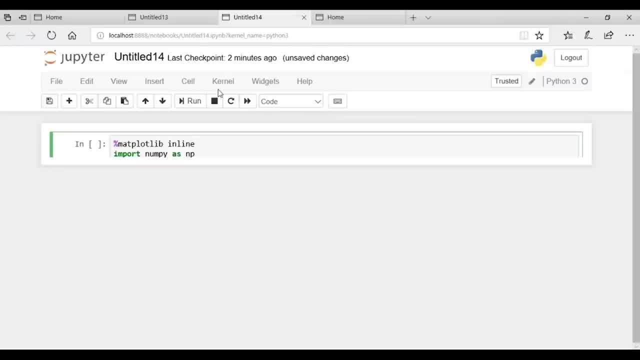 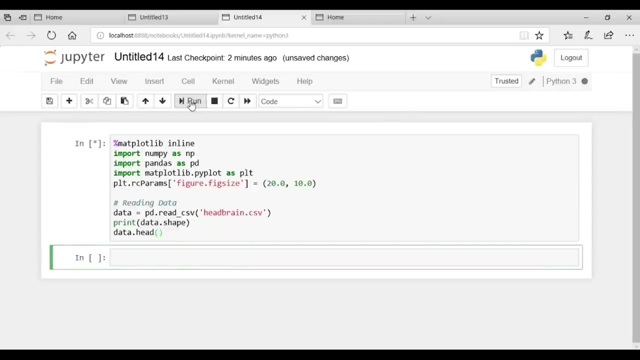 as as pd and matplotlib, and from matplotlib we are importing pi plot of that as plt. all right, next we'll import our data head brain dot csv and store it in the data variable. let's execute the run button and see the output. so this asterisk symbol. it symbolizes that it's still executing. 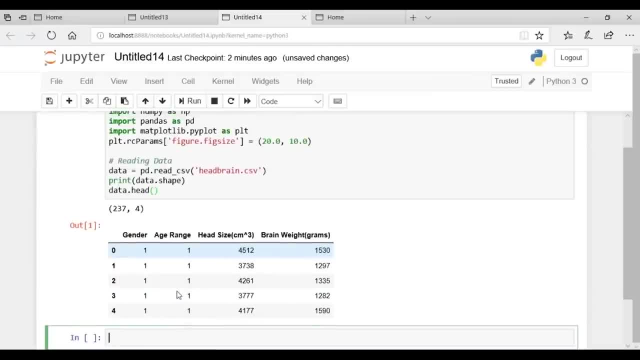 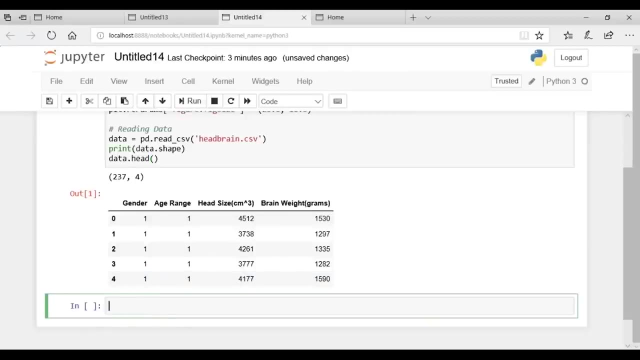 so there's a output. our data set consists of 237 rows and four columns. we have columns as gender, age range, head size in centimeter cube and brain weights in gram fine. so this is our sample data set. this is how it looks. it consists of all these data set, so now, 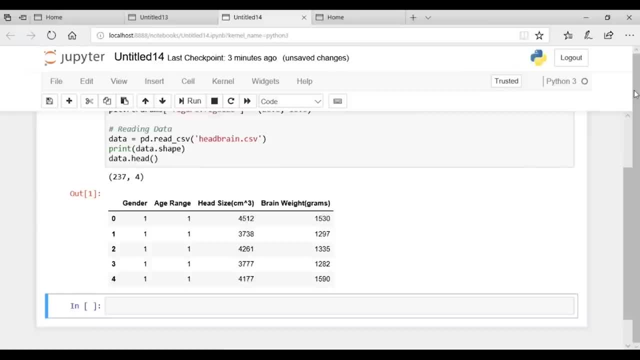 that we have imported our data. so, as you can see, there are 237 values in the training set, so we can find a linear relationship between the head size and the brain weights. so now what we'll do? we'll collect x and y. the x would consist of the head size values and the y would consist of 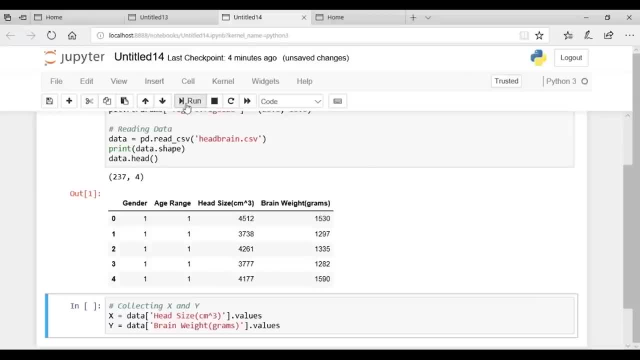 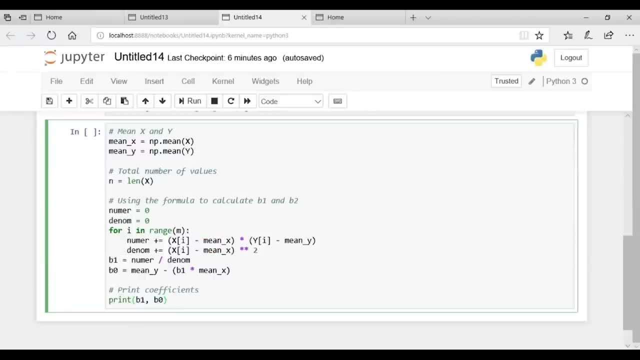 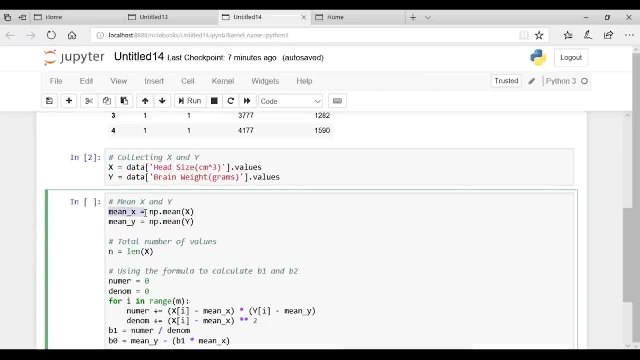 brain weight values. so collecting x and y, let's execute the run. i'm done. next, what we'll do: we need to find the values of b1 or b naught, or you can say m and c. so we'll need the mean of x and y values first of all. what we'll do: we'll calculate the mean of x and y, so mean x. 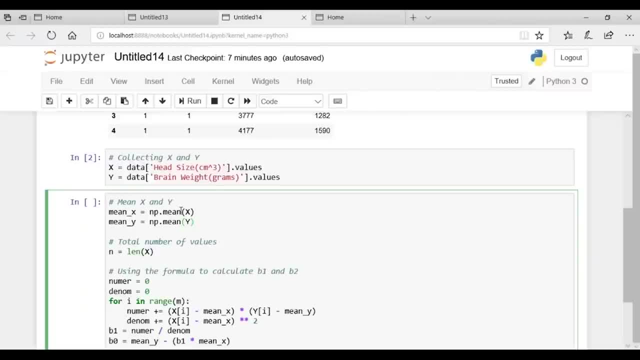 equal np dot mean x. so mean is a predefined function of numpy. similarly, mean underscore y equal np dot mean of y. so what it will return? it will return the mean values of y. next we'll check the total number of values. so m equal length of x. all right, 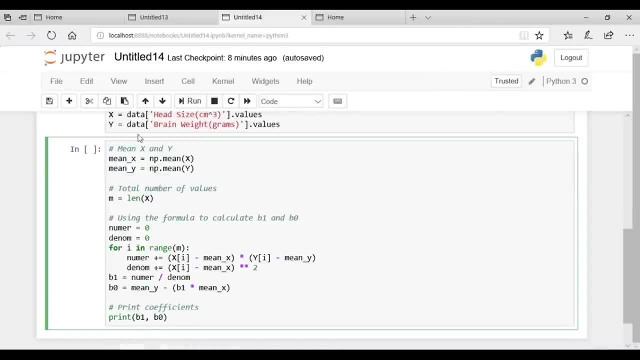 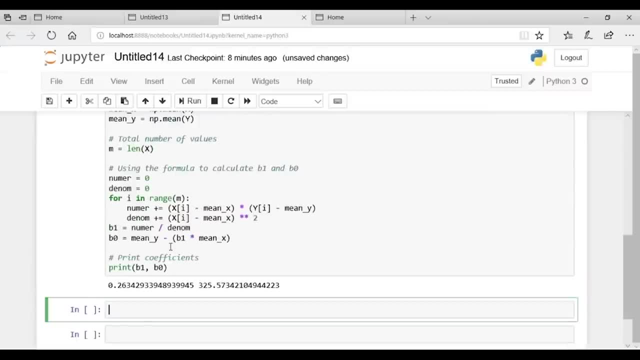 then we'll use the formula to calculate the values of b1 and b, naught or mnc. all right, let's execute the run button and see what is the result. so, as you can see here on the screen, we have got b1 as 0.263 and b naught as 325.57. all right, so now that we have our coefficient. so, comparing it with the 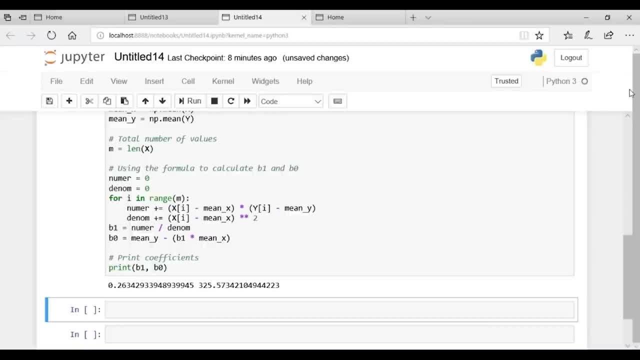 equation y equal mx plus c. you can say that brain weight equals 0.263 multiplied by head size plus five point five seven. so you can say that the value of m here is 0.263 and the value of c here is 325.57. all right, so this is our linear model. now let's plot it and see graphically. 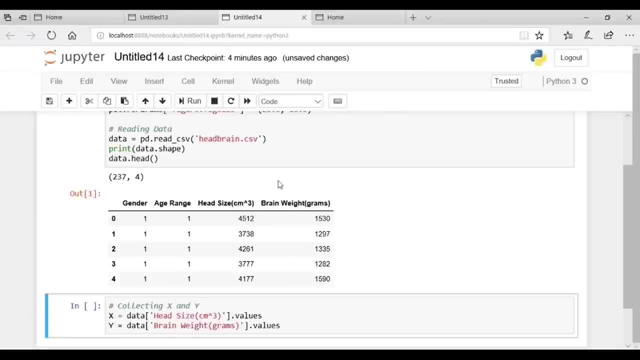 so we can find a linear relationship between the head size and the brain weights. So now, what we'll do will collect X and Y. the X would consist of the head size values and the Y would consist of brain weight values. So collecting X and Y. 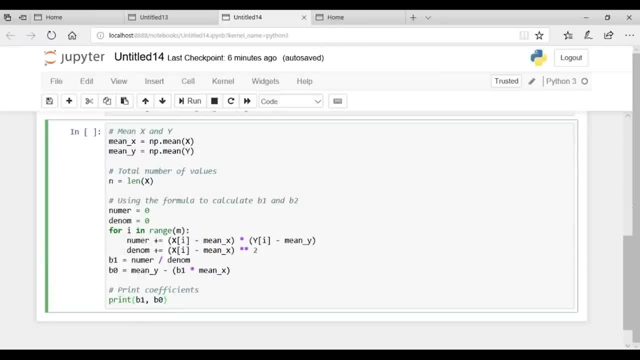 Let's execute the run Done. Next, what we'll do? we need to find the values of B1 or B naught, or you can say M and C, So we'll need the mean of X and Y values First of all. what we'll do will calculate the mean of X and 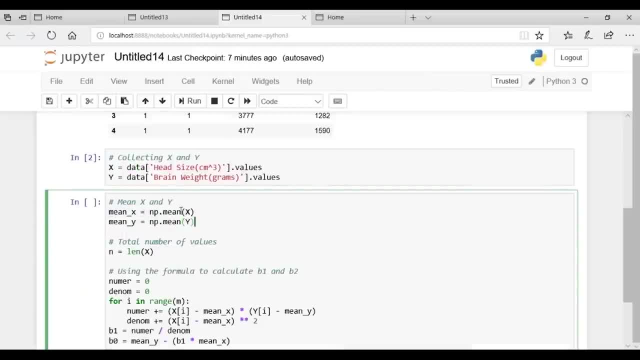 Y. So mean X equal NP dot mean. X. So mean is a predefined function of number. Similarly, mean underscore Y equal NP dot mean of Y. So what it will return if we return the mean values of Y. next We'll check the total number of values. 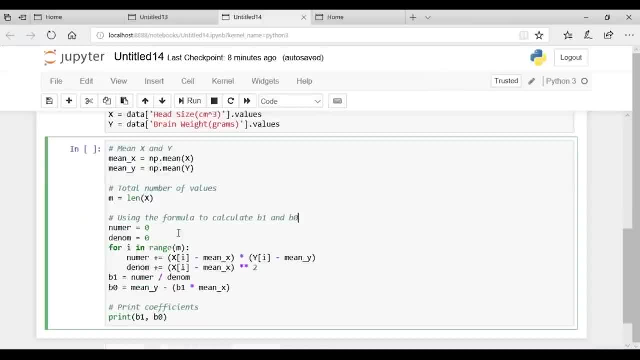 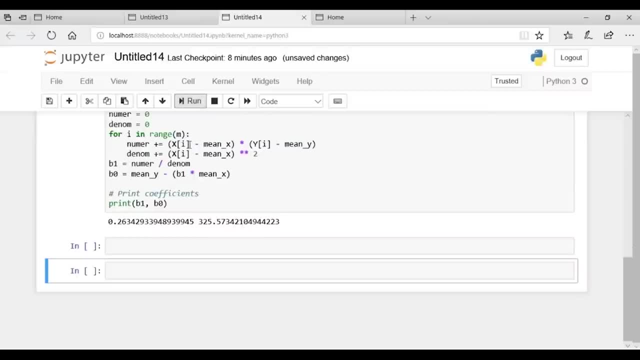 So M equal length of X. All right, then we'll use the formula to calculate the values of B1 and B, naught or MNC. All right, let's execute the run button and see what is the result. So, as you can see here on the screen, we have got B1 as 0.263. 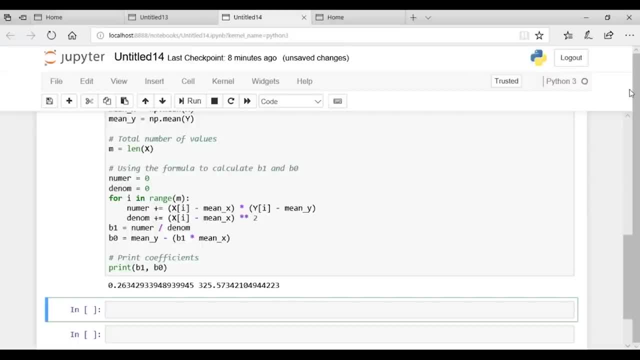 and B naught as 325.57.. All right, So now that we have our coefficient. so, comparing it with the equation Y equal MX plus C, you can say that brain weight equals 0.263 multiplied by head size plus 325.57. 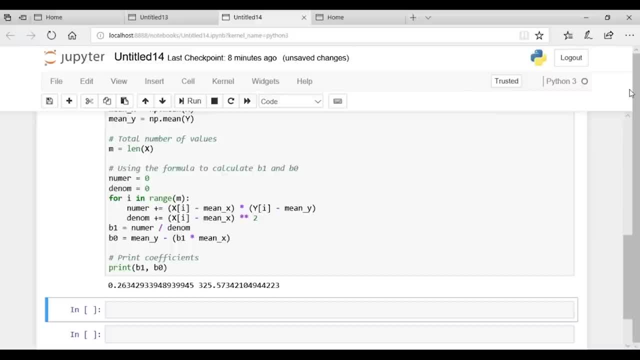 So you can say that the value of M here is 0.263 and the value of C here is 325.57.. All right, so there's our linear model. Now let's plot it and see graphically, Let's execute it. 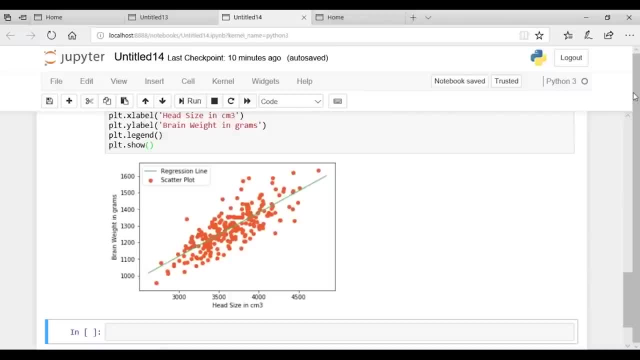 So this is how our plot looks like. this model is not so bad, but we need to find out how good our model is. So, in order to find it, There are many methods like root mean square method, the coefficient of determination or the R square method. 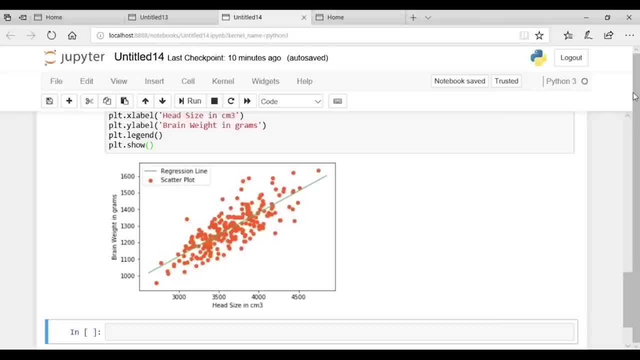 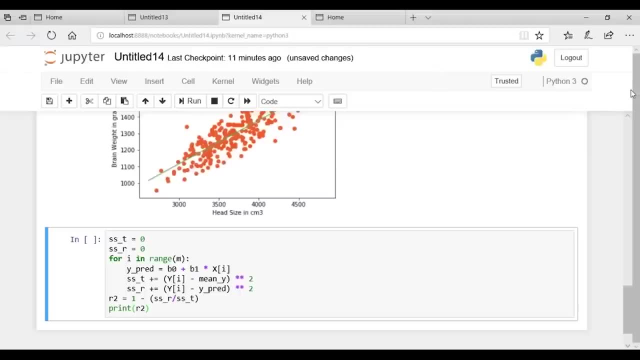 So in this tutorial I have told you about R square method, So let's focus on that and see how good our model is. So let's calculate the R square value. All right here. SS underscore T is the total sum of square. SS underscore R is the total sum of square of residuals. 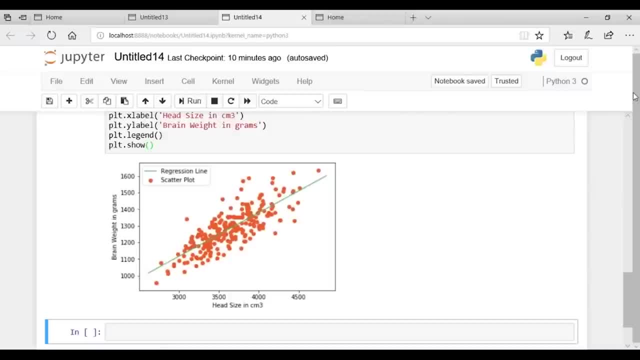 let's execute it. so this is how our plot looks like. this model is not so bad, but we need to find out how good our model is. so in order to find it, there are many methods like root mean square method, the coefficient of determination or the r squared method. 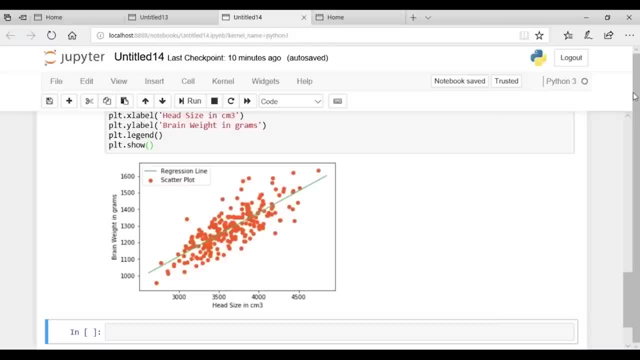 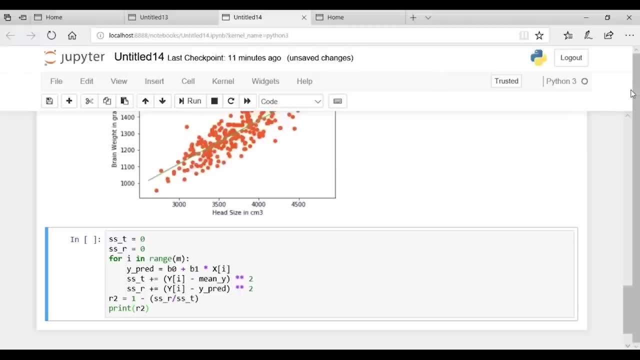 So in this tutorial I have told you about R square method, So let's focus on that and see how good our model is. So let's calculate the R square value. All right here. SS underscore T is the total sum of square. SS underscore R is the total sum of square of residuals. 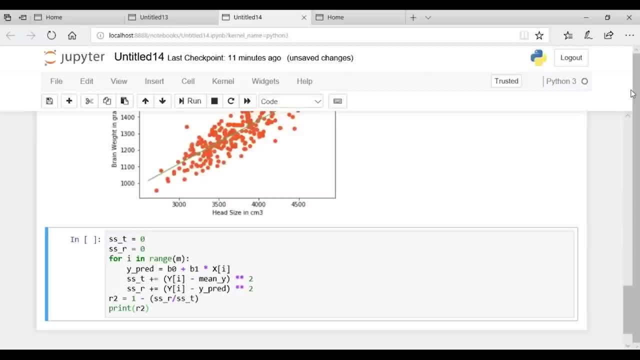 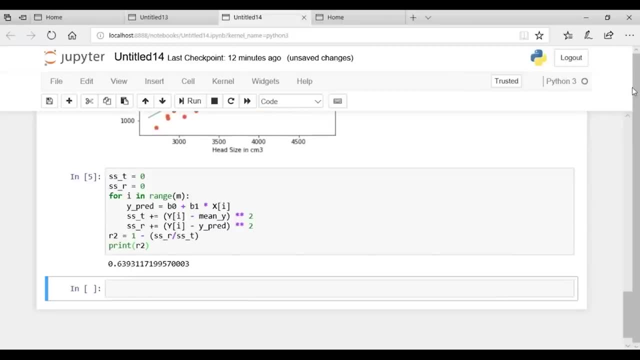 and R square, as the formula is 1 minus total sum of squares upon total sum of square of residuals. All right. next, when you execute it, you will get the value of R square as 0.63.. Which is pretty, very good Now that you have implemented simple linear regression model. 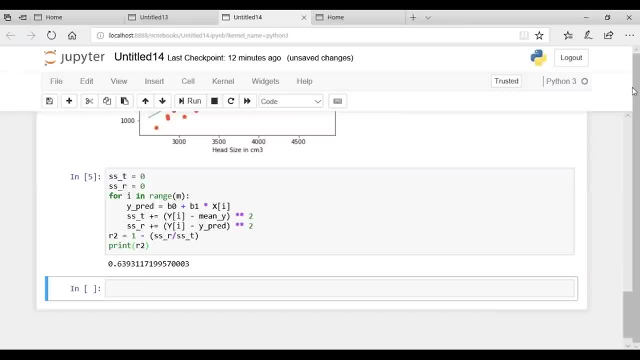 using least square method. Let's move on and see how will you implement the model using machine learning library called scikit-learn. All right, So this scikit-learn is a simple machine learning library in Python. building machine learning model are very easy. 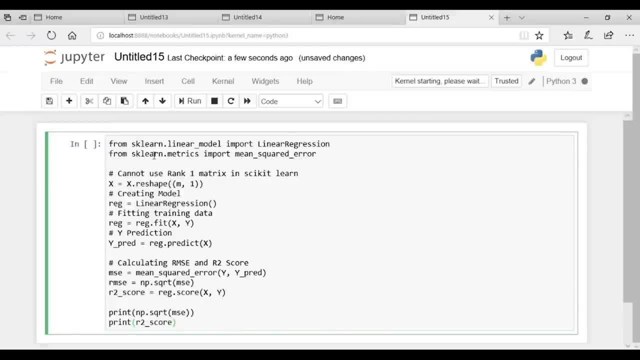 using scikit-learn. So suppose this is your Python code. So, using the scikit-learn libraries, your code shortens to this length. All right, So let's execute the run button and see you'll get the same R2 score. 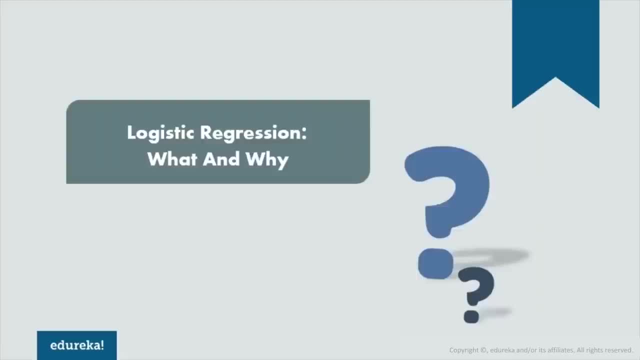 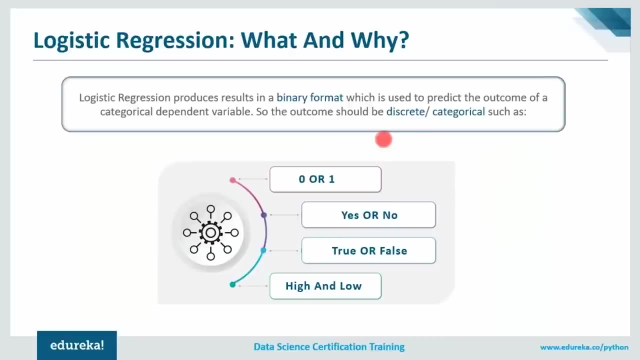 So today we'll be discussing logistic regression. So let's move forward and understand the what and why of logistic regression. Now. this algorithm is most widely used when the dependent variable, or you can say the output, is in the binary format. So here you need to predict the outcome. 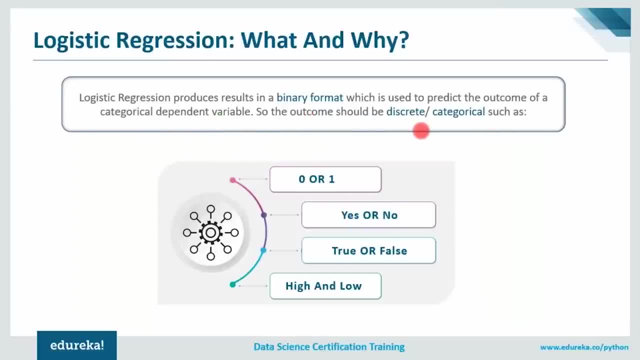 of a categorical dependent variable. So the outcome should be always discrete or categorical in nature. Now by discrete I mean the value should be binary, or you can say you just have two values. It can either be 0 or 1.. It can either be yes or no, either be true or false. 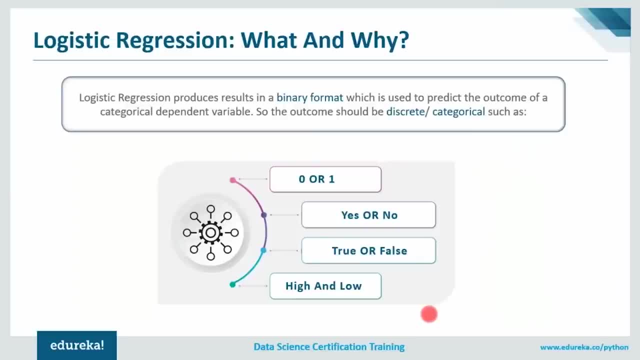 or high or low, So only these can be the outcomes. So the value which you need to predict should be discrete, or you can say categorical in nature, Whereas in linear regression we have the value of Y or you can say the value you need. 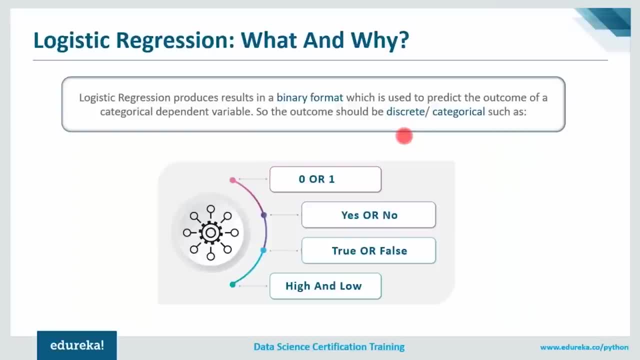 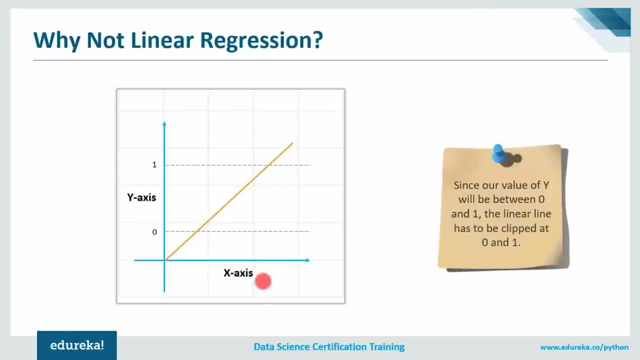 to predict is in a range. So that is how there is a difference between linear regression and logistic regression. Now you must be having question: Why not linear regression? now, guys, in linear regression, the value of Y, or the value which you need to predict, is in a range. 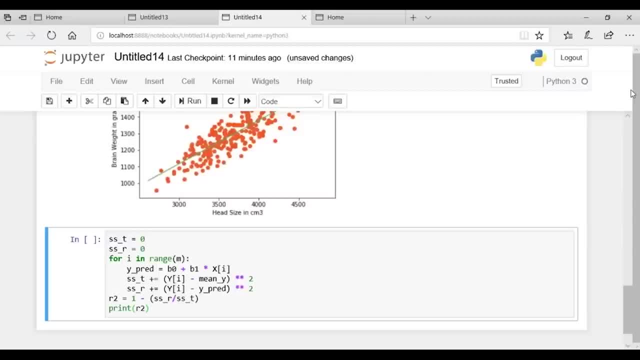 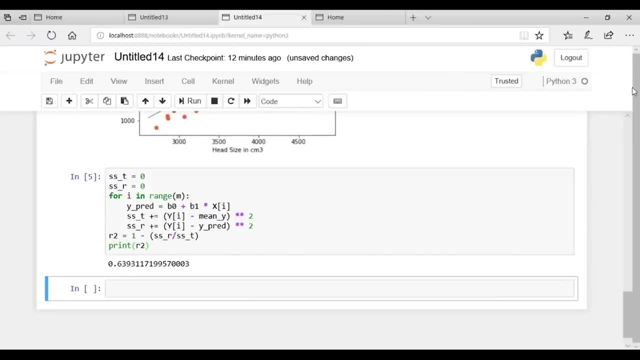 and R square, as the formula is 1 minus total sum of squares upon total sum of square of residuals. All right. next, when you execute it, you'll get the value of R square as 0.63, which is pretty, very good Now that you have implemented simple linear regression model. 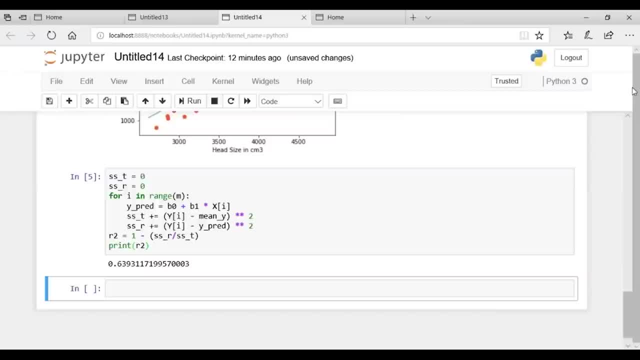 using least square method. Let's move on and see how will you implement the model using machine learning library called scikit-learn. All right, So this scikit-learn is a simple machine learning library in Python. building machine learning model are very easy. 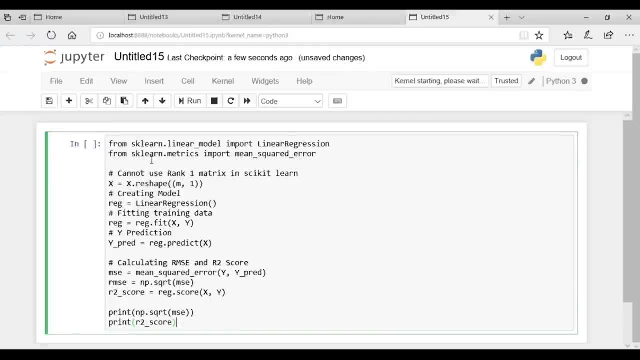 using scikit-learn. So suppose there's a Python code. So, using the scikit-learn Learn libraries, your code shortens to this length. All right, so let's execute the run button and see you'll get the same R2 score. 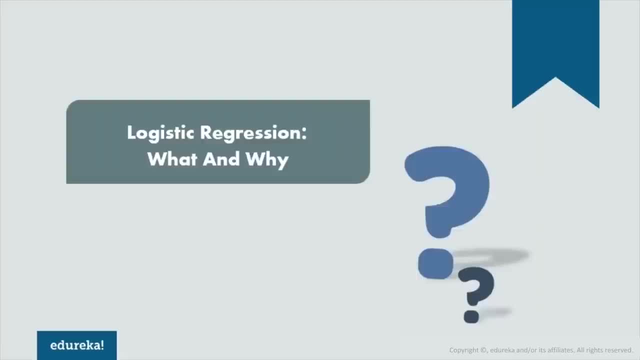 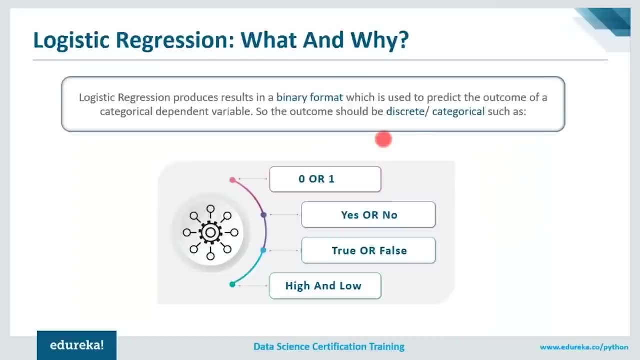 So today we'll be discussing logistic regression. So let's move forward and understand the what and why of logistic regression. Now. this algorithm is most widely used when the dependent variable, or you can say the output, is in the binary format. So here you need to predict the outcome. 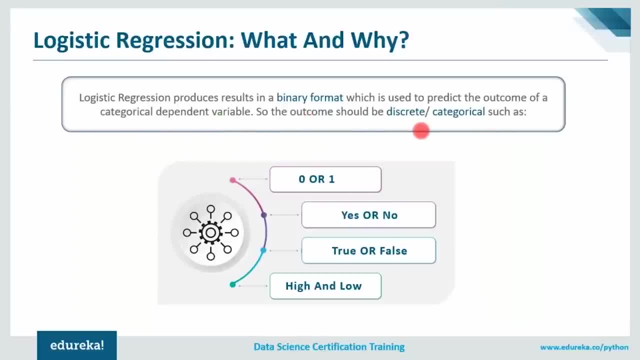 of a categorical dependent variable. So the outcome should be always discreet or categorical in nature. now by discrete, I mean the value should be binary, or you can say you just have two values. It can either be 0 or 1. it can either be yes. 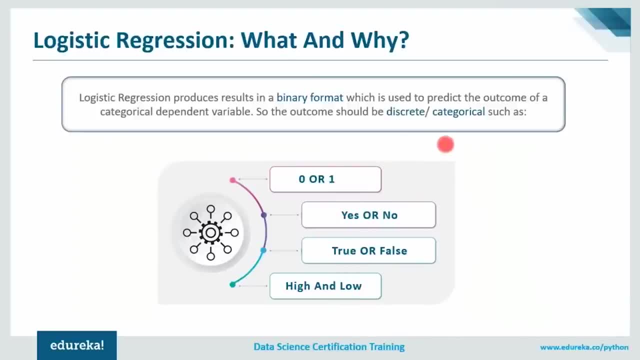 or no, either be true or false, or high or low, So only these can be the outcomes. So the value which you need to predict should be discreet, or, you can say, categorical in nature. Whereas in linear regression we have the value of Y, or you can say the value need to predict is in a range. 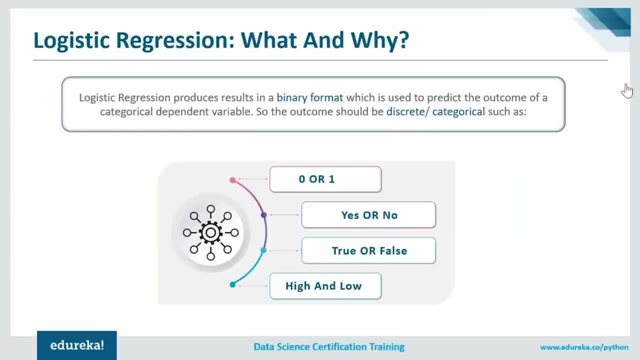 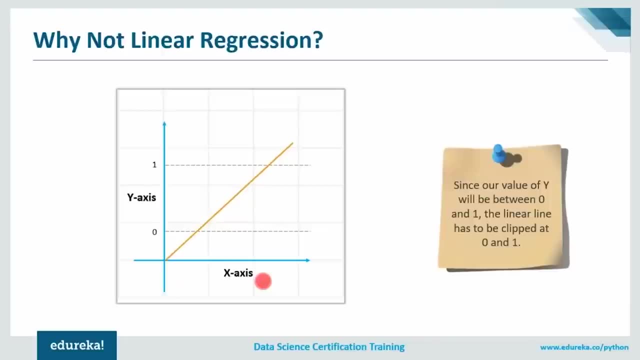 So that is how there's a difference between linear regression and logistic regression. We must be having question: Why not linear regression? now, guys, in linear regression, the value of Y, or the value which you need to predict, is in a range, But in our case, as in the logistic regression, 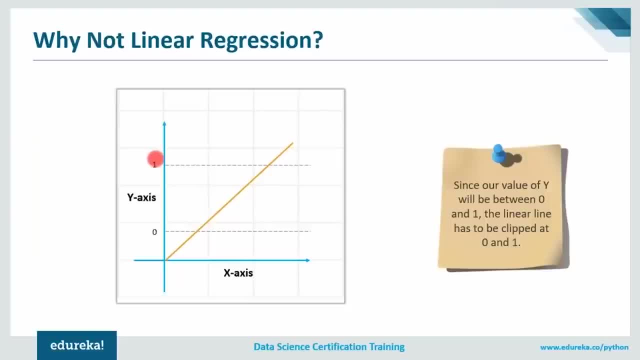 we just have two values. It can be either 0 or it can be one. It should not entertain the values which is below 0 or above 1.. But in linear regression we have the value of Y in the range. So here, in order to implement logistic regression, 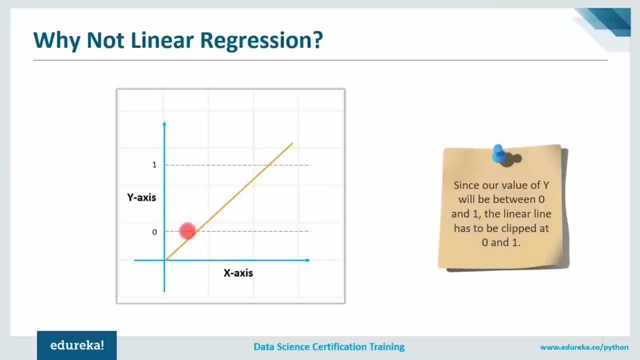 we need to clip this part, So we don't need the value that is below 0, or we don't need the value which is above 1.. So, since the value of Y will be between only 0 and 1, that is the main rule of logistic regression. 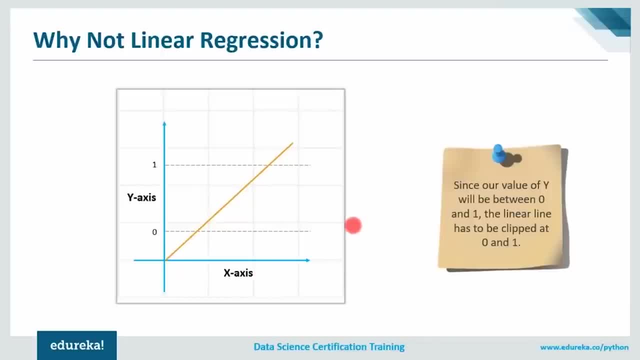 but in our case, as in the logistic regression, we just have two values. It can be either 0 or it can be 1. it should not entertain the values which is below 0 or above 1, but in linear regression we have the value of Y in the range. 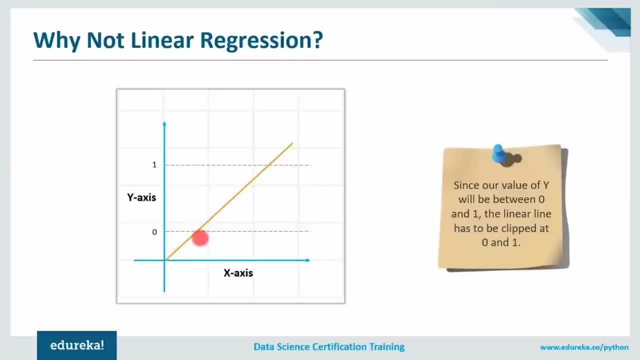 So here, in order to implement logistic regression, we need to clip this part, So we don't need the value that is below 0, or we don't need the value which is above 1.. So, since the value of Y will be between only 0 and 1, 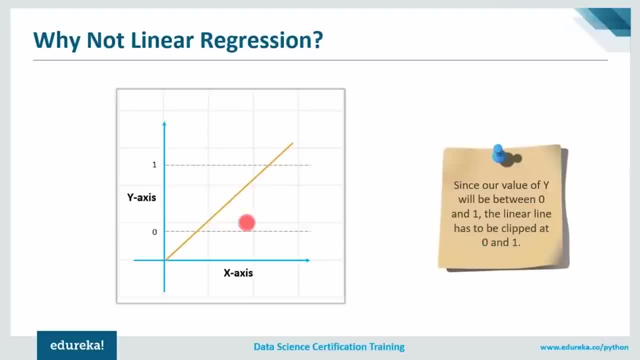 that is the main rule of logistic regression. The linear line has to be clipped at 0 and 1.. Now, once we clip this graph, it would look somewhat like this: So here you are getting the curve, which is nothing but three different straight lines. 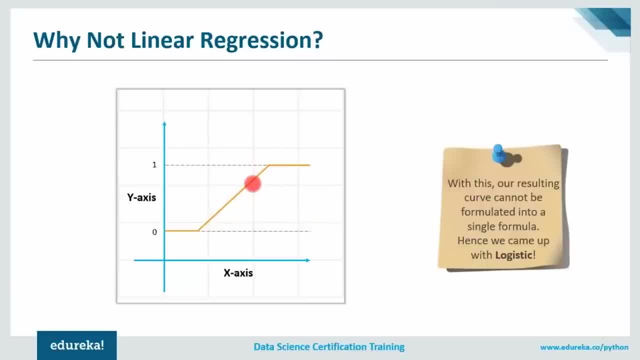 So here we need to make a new way to solve this problem. So this has to be formulated into equation, and hence we come up with logistic regression. So here the outcome is either 0 or 1, which is the main rule of logistic regression. 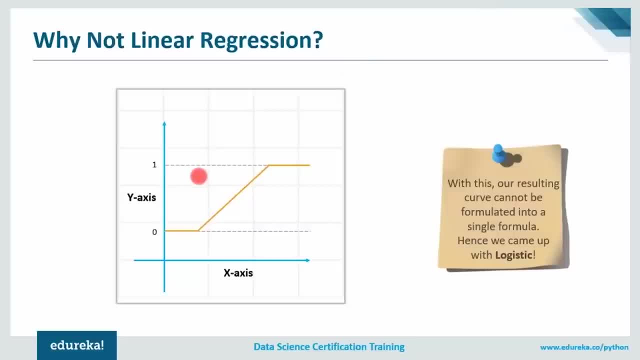 So with this, a resulting curve cannot be formulated. So hence our main aim, to bring the values to 0 and 1, is fulfilled. So that is how we came up with logistic regression Now here. once it gets formulated into an equation, it looks somewhat like this: 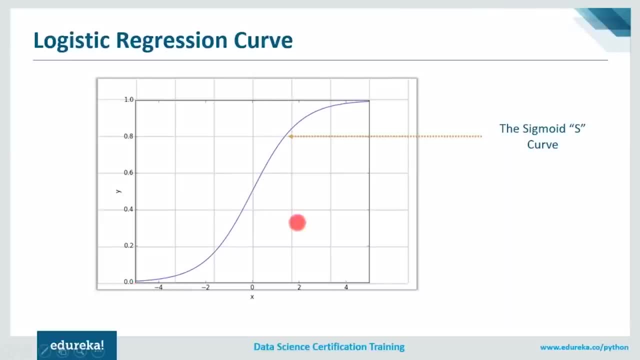 So, guys, this is nothing but a S curve, or you can say the sigmoid curve, or sigmoid function curve. So this sigmoid function basically converts any value from minus infinity to infinity, to your discrete values which a logistic regression wants, or you can say the values which are in binary format. 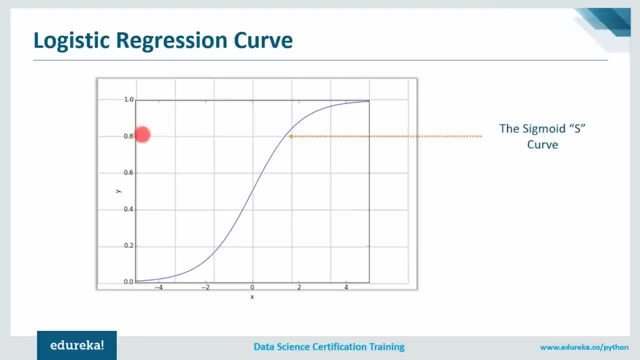 either 0 or 1.. So if you see, here the values are either 0 or 1 and this is nothing but just a transition of it. But, guys, there's a catch over here. So let's say I have a data point that is 0.8.. 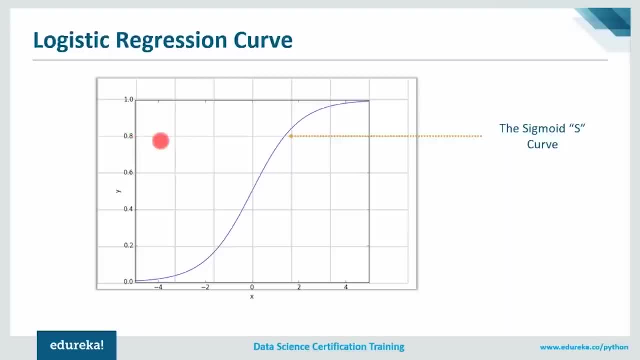 Now, how can you decide whether your value is 0 or 1? now, here you have the concept of threshold, which basically divides your line. So here threshold value basically indicates the probability of either winning or losing. So here by winning I mean the values equals to 1, and by losing 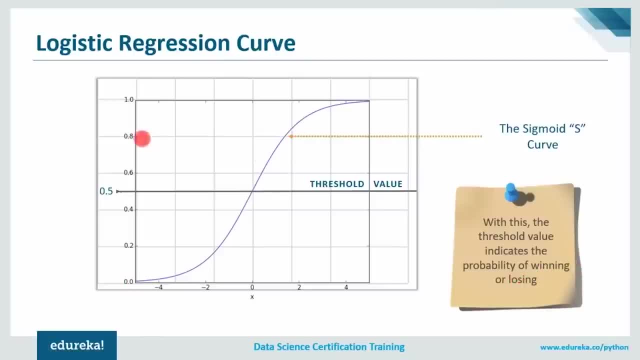 I mean the values equals to 0. but how does it do that? Let's say I have a data point which is over here. Let's say my cursor is at 0.8.. So here I'll check whether this value is less than my threshold value. 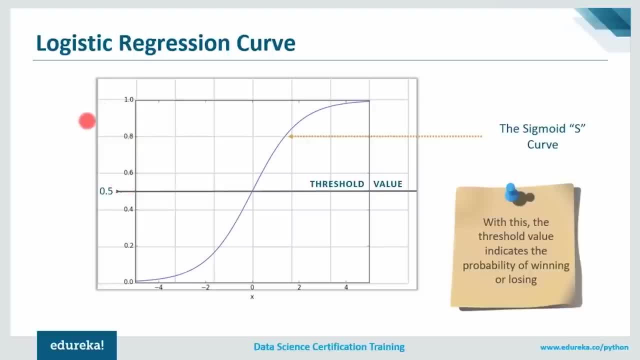 or not. Let's say, if it is more than my threshold value, it should give me the result as 1, if it is less than that, then should give me the result as 0.. So here my threshold value is 0.5.. 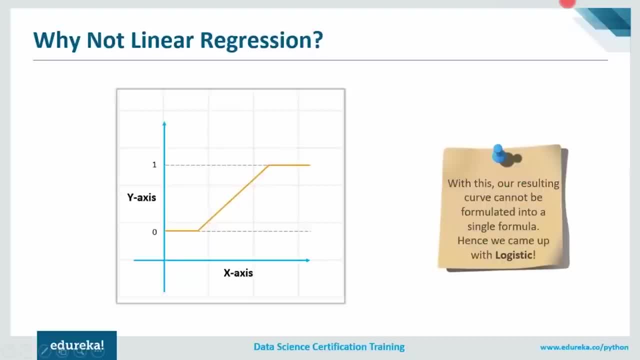 The linear line has to be clipped at 0 and 1.. Now, once we clip this graph, it would look somewhat like this: So here you are getting the curve, which is nothing but three different straight lines. So here we need to make a new way to solve this problem. 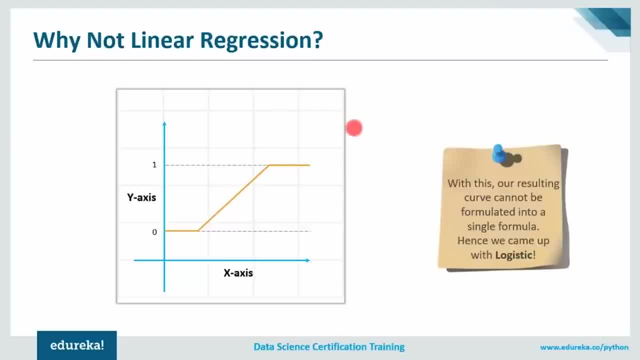 So this has to be formulated into equation, and hence we come up with logistic regression. So here the outcome is either 0 or 1, which is the main rule of logistic regression. So with this our resulting curve cannot be formulated. So hence our main aim, to bring the values to 0 and 1, is fulfilled. 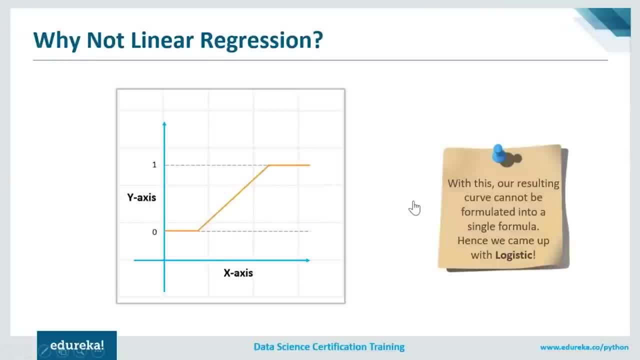 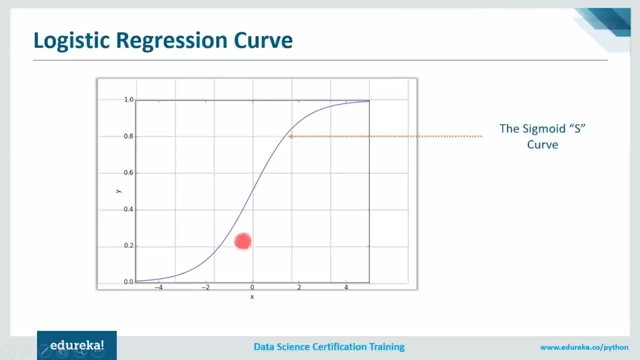 So that is how we came up with logistic regression. Now here, once it gets formulated into an equation, it looks somewhat like this: So, guys, this is nothing but a S curve, or you can say the sigmoid curve, or sigmoid function curve. So this sigmoid function basically converts any value. 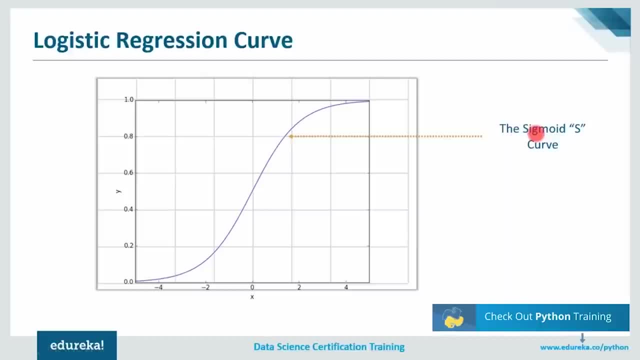 from minus infinity to infinity, to your discrete values, which a logistic regression wants. or you can say the values which are in binary format, either 0 or 1.. So if you see, here the values are either 0 or 1 and this is nothing but just a transition of it. 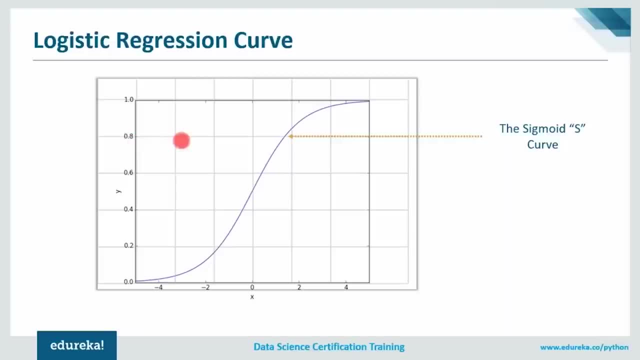 But, guys, there's a catch over here. So let's say, I have a data point that is 0.8.. Now how can you decide whether your value is 0 or 1? Now, here you have the concept of threshold, which basically divides your line. 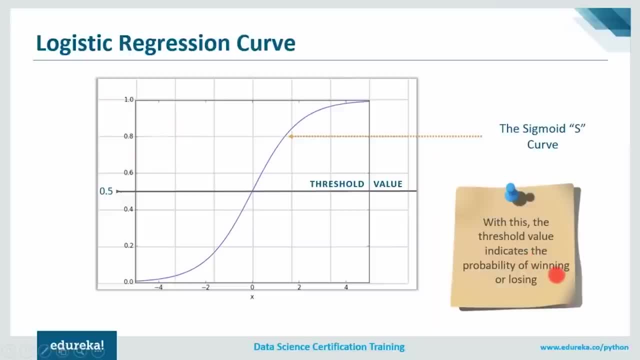 So here threshold value basically indicates the probability of either winning or losing. So here, by winning I mean the values equals to 1, and by losing I mean the values equals to 0. But how does it do that? Let's say I have a data point which is over here. 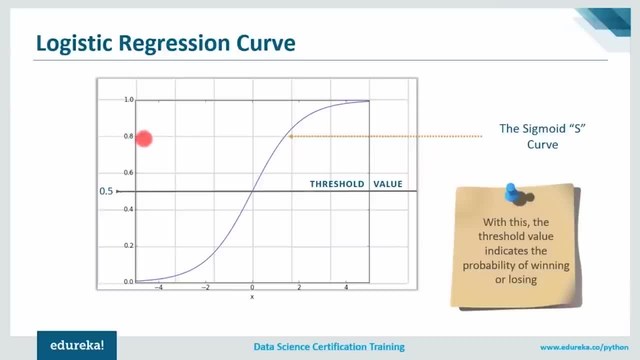 Let's say, my cursor is at 0.8.. So here I'll check whether this value is less than my threshold value or not. Let's say, if it is more than my threshold value, it should give me the result as 1.. 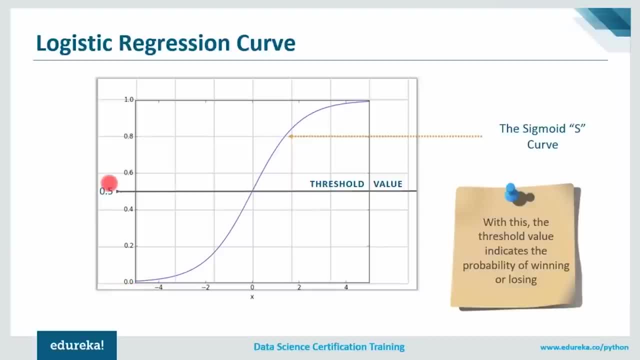 If it is less than that, then should give me the result as 0.. So here my threshold value is 0.5.. Now I need to define that. if my value, let's say 0.8.. It is more than 0.5, then the value shall be rounded off to 1. 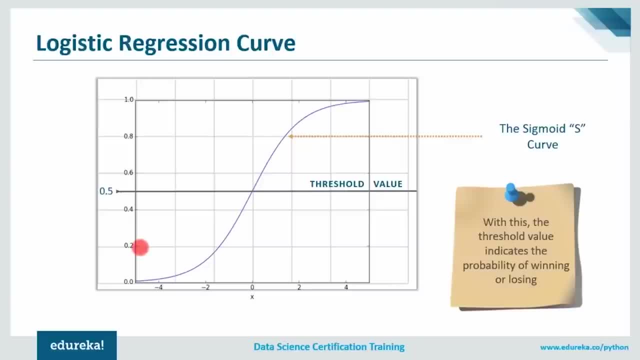 and let's say if it is less than 0.5.. Let's say I have a values 0.2, then should reduce it to 0. So here you can use the concept of threshold value to find your output. So here it should be discrete. 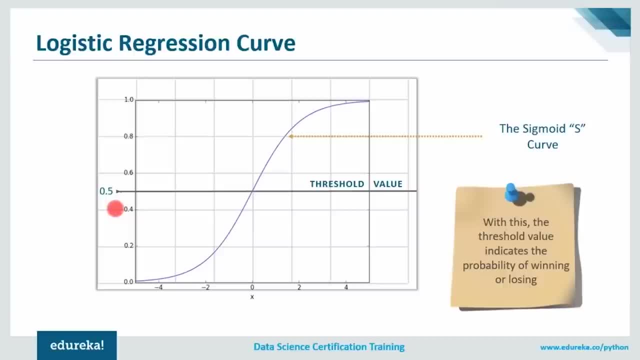 Now I need to define if my value- let's say 0.8. It is more than 0.5. Then the value shall be rounded off to 1. and let's say if it is less than 0.5.. Let's say I have a values 0.2, then should reduce it to 0.. 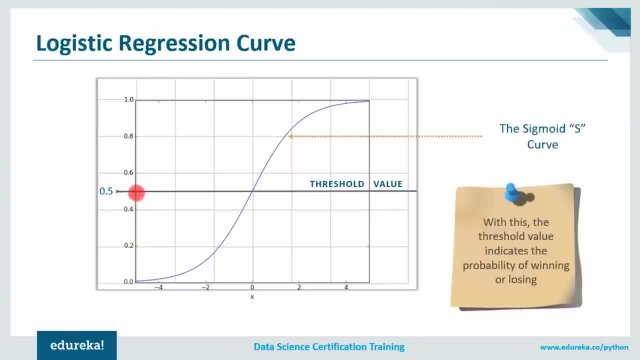 So here you can use the concept of threshold value to find your output. So here it should be discrete, It should be either 0 or it should be 1.. So I hope you caught this curve of logistic regression. So, guys, this is the sigmoid S curve. 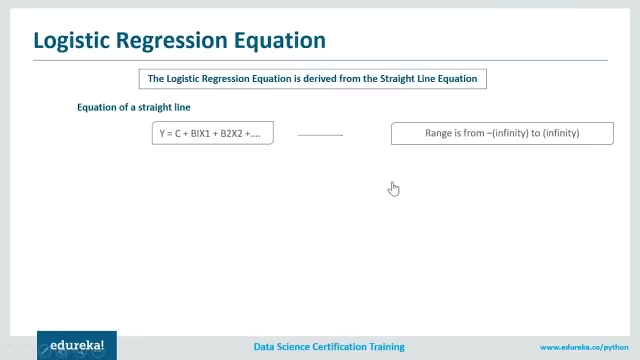 So to make this curve we need to make an equation, So let me address that part as well. So let's see how an equation is formed to imitate this functionality. So over here we have an equation of a straight line, which is y. 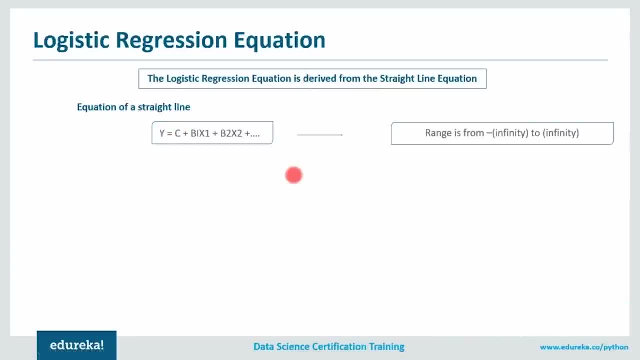 is equals to MX plus C. So in this case I just have only one independent variable. but let's say, if we have many independent variable, then the equation becomes m1x1 plus m2x2 plus m3x3 and so on till mnxn. 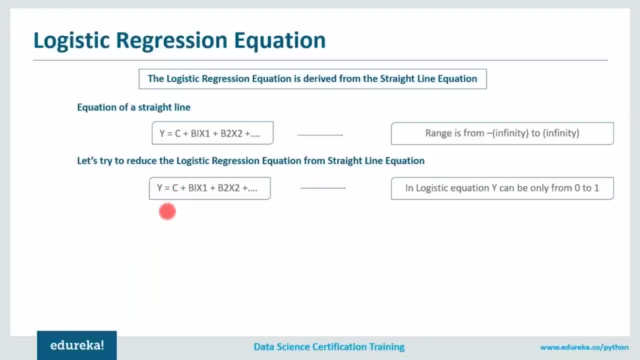 Now let us put in b and x, So here the equation becomes: y is equals to b1x1 plus b2x2 plus b3x3, and so on till bnxn plus C. So, guys, your equation of the straight line has a range from minus. 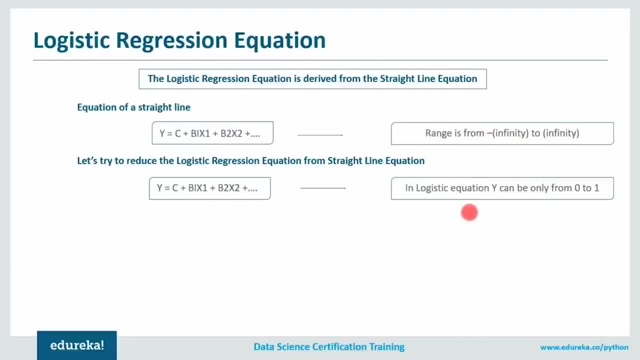 infinity to infinity. But in our case, or you can say in logistic equation the value which we need to predict, or you can say the y value. it can have the range only from 0 to 1.. So in that case we need to transform this equation. 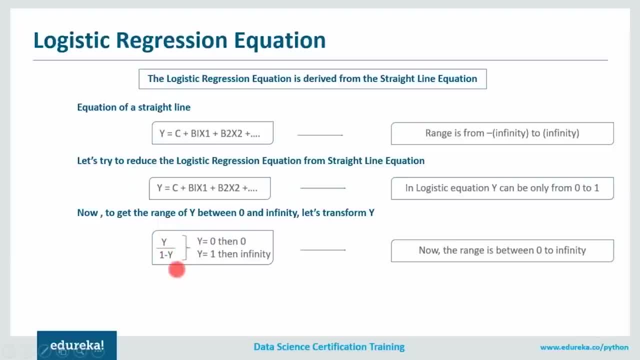 So to do that, what we had done, we have just divide the equation by 1 minus y, So now our y is equals to 0. So 0 over 1 minus 0, which is equals to 1.. So 0 over 1 is again 0, and if we take y is equals to 1, then 1 over 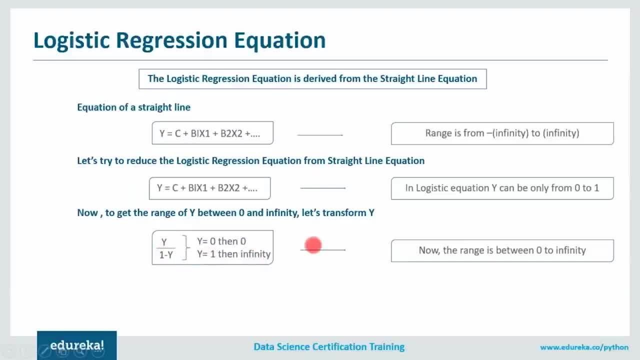 1 minus 1, which is 0. So 1 over 0 is infinity. So here my range is now between 0 to infinity. But again, we want the range from minus infinity to infinity. So for that, what we'll do will have the log of this equation. 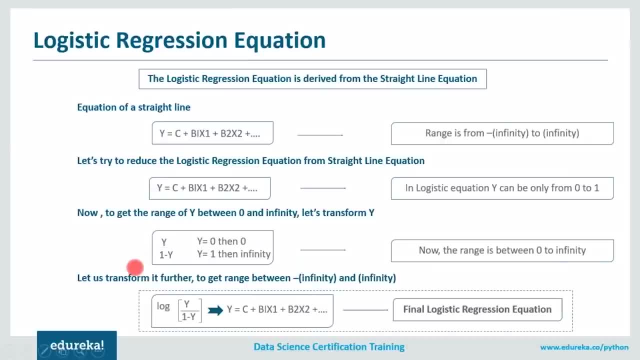 So let's go ahead and have the logarithmic of this equation. So here we have this. transform it further to get the range between minus infinity to infinity. So over. here we have log of y over 1 minus 1, and this is your final. 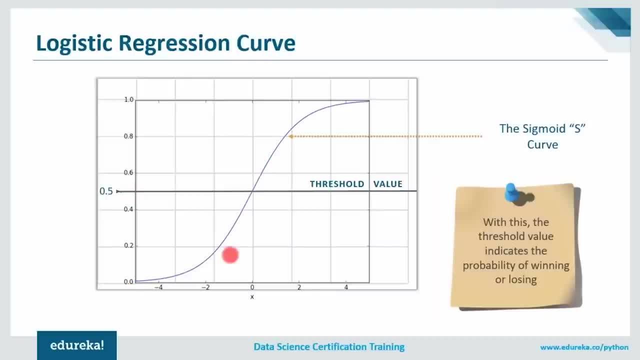 It should be either 0 or it should be 1.. So I hope you caught this curve of logistic regression. So, guys, this is the sigmoid S curve. So to make this curve we need to make an equation. So let me address that part as well. 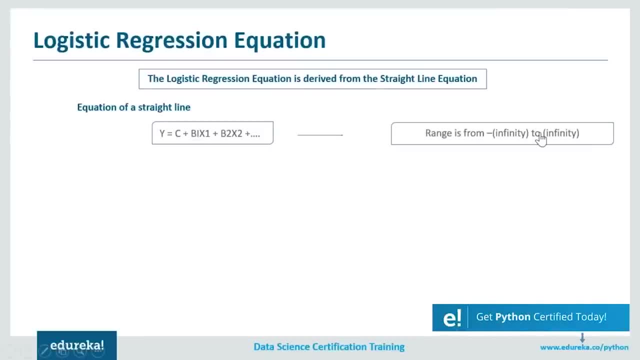 So let's see how an equation is formed to imitate this functionality. So over here we have an equation of a straight line which is: y is equals to MX plus C. So in this case I just have only one independent variable. but let's say, if we have many independent variable. 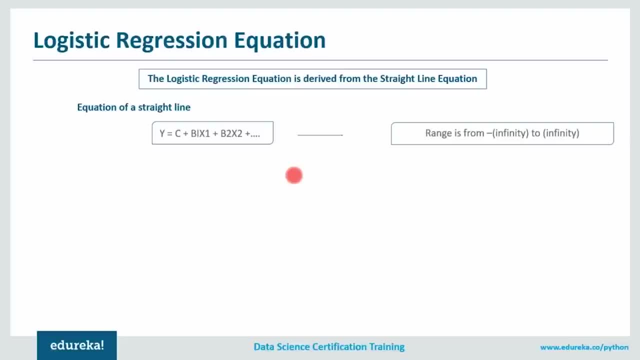 then the equation becomes: m1 x1 plus m2 x2 plus m3 x3, and so on till mn xn. Now let us put in b and x, So here the equation becomes: y is equals to b1 x1 plus b2 x2 plus b3 x3. 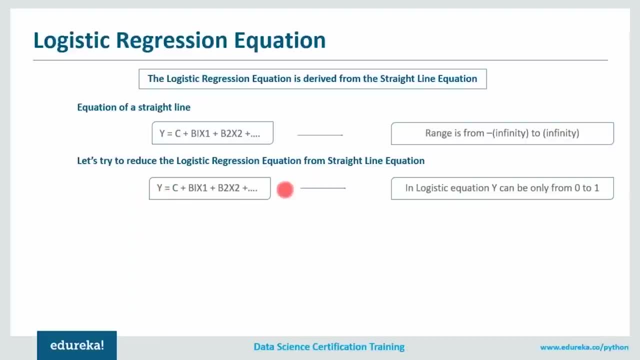 and so on, till bn, xn plus C. So, guys, your equation of the straight line has a range from minus infinity to infinity. But in our case, or you can say logistic equation, the value which we need to predict, or you can say the y value. 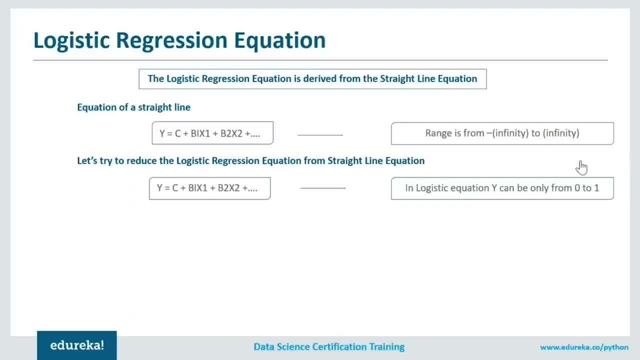 it can have the range only from 0 to 1.. So in that case we need to transform this equation. So to do that what we had done, we have just divide the equation by 1 minus y, So now y is equals to 0.. 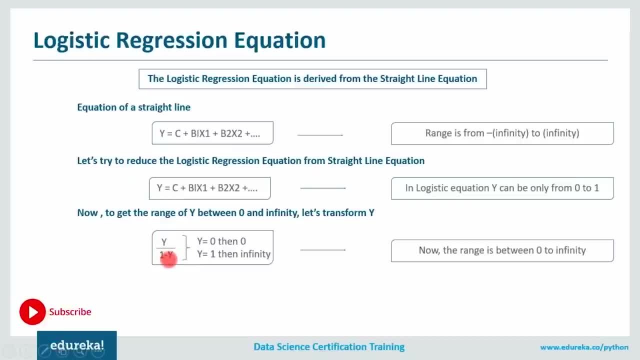 So 0 over 1 minus 0 is just equals to 1.. So 0 over 1 is again 0, and if we take y is equals to 1, then 1 over 1 minus 1, which is 0. So 1 over 0 is infinity. 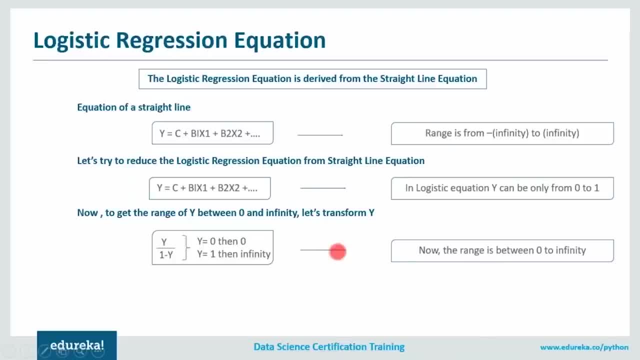 So here, my range is now between 0 to infinity, But again, we want the range from minus infinity to infinity. So for that, what we'll do will have the log of this equation. So let's go ahead and have the logarithmic of this equation. 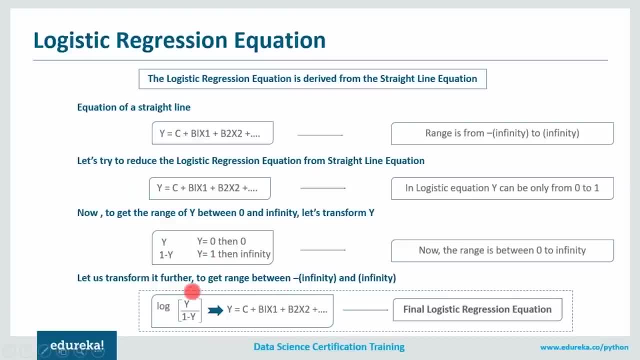 So here we have this. transform it further to get the range between minus infinity to infinity. So over here we have log of y over 1 minus 1 and this is your final logistic regression equation. So, guys, don't worry, You don't have to write this formula or memorize this formula in Python. 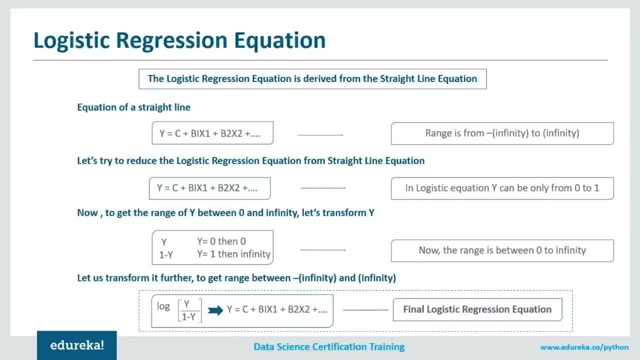 You just need to call this function, which is logistic regression, and everything will be automatically for you. So I don't want to scare you with the maths and the formulas behind it, but it's always good to know how this formula was generated. So I hope you guys are clear with how logistic regression comes into the picture. 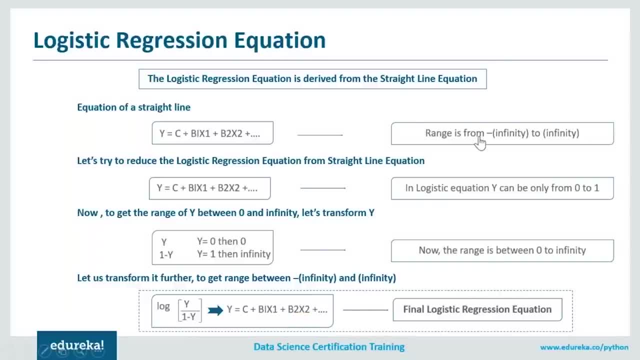 logistic regression equation. So, guys, don't worry, You don't have to write this formula or memorize this formula In Python. you just need to call this function, which is logistic regression, and everything will be automatically for you. So I don't want to scare you with the maths and the formulas behind. 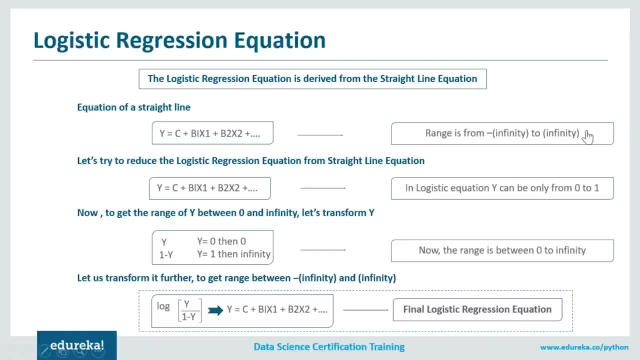 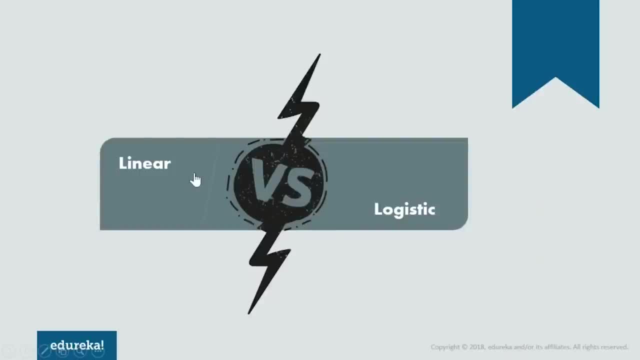 it, but it's always good to know how this formula was generated. So I hope you guys are clear with how logistic regression comes into the picture. Let's let us see What are the major differences between linear regression versus logistic regression. Now, first of all, in linear regression we have the value of y. 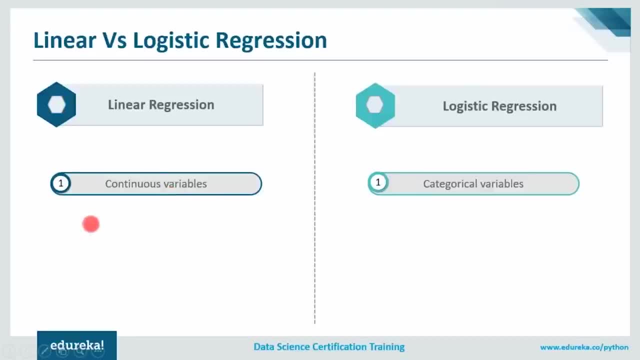 as a continuous variable or the variable which we need to predict our continuous nature, Whereas in logistic regression we have the categorical variable. So here the value which you need to predict should be discrete in nature. It should be either 0 or 1, or it should have just two values to. 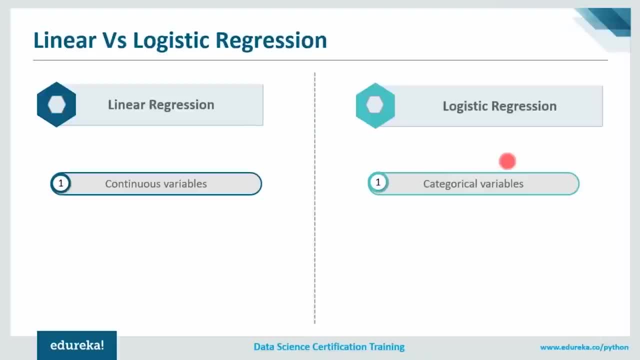 it, For example, whether it is raining or it is not raining. Is it Humid outside or it is not humid outside? Now, does it going to snow or it is not going to snow? So these are the few example where you need to predict where the 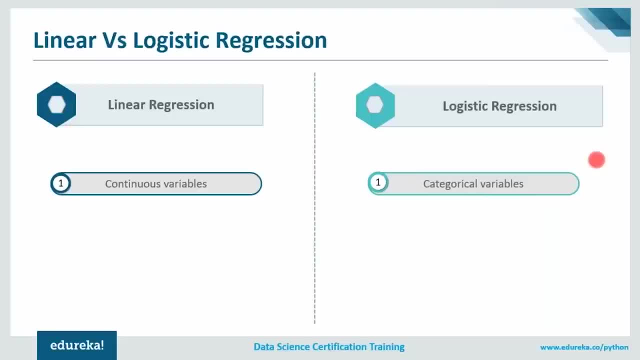 values are discrete, or you can just predict whether this is happening or not. Next, linear regression solves your regression problems. So here you have a concept of independent variable and a dependent variable. So here you can calculate the value of y which you need to predict. 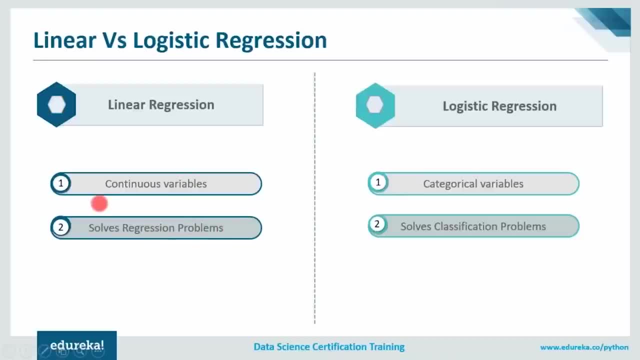 using the value of x. So here your y variable, or you can say the value that you need to predict, are in a range, But whereas in logistic regression you have discrete values. So logistic regression basically solves your classification problem. So it can basically classify it and it can just give you result. 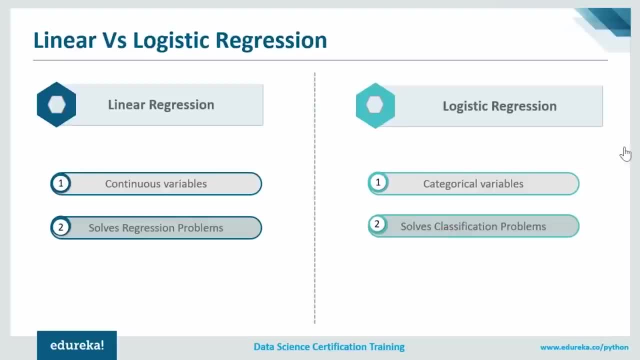 whether this event is happening or not. So I hope it is pretty much clear till now. Next, in linear regression, the graph that you have seen is a straight line graph, So over here you can calculate the value of y with respect to the. 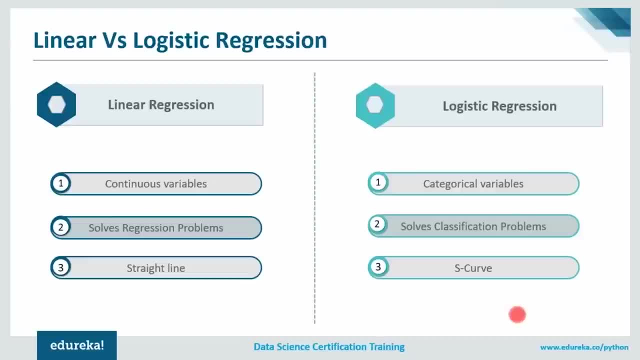 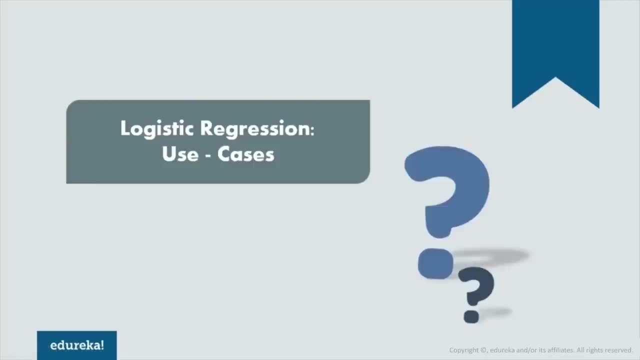 value of x, Whereas in logistic regression, the curve that we got was a s curve, or you can say the sigmoid curve. So using the sigmoid function, you can predict your y values Moving ahead. Let us see the various use cases where, in logistic regression, 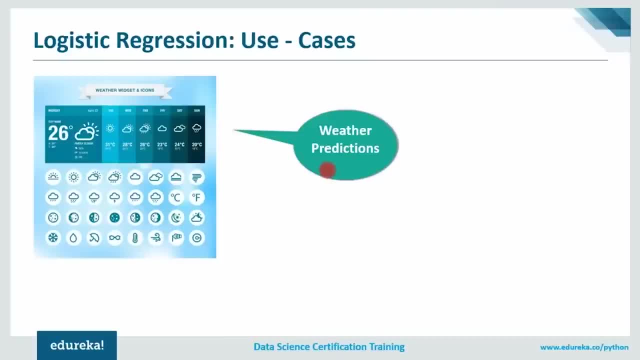 is implemented in real life. So the very first is weather prediction. Now, logistic regression helps you to predict your weather. For example, it is used to predict whether it is raining or not, whether it is sunny, Is it cloudy or not. So all these things can be predicted using logistic regression. 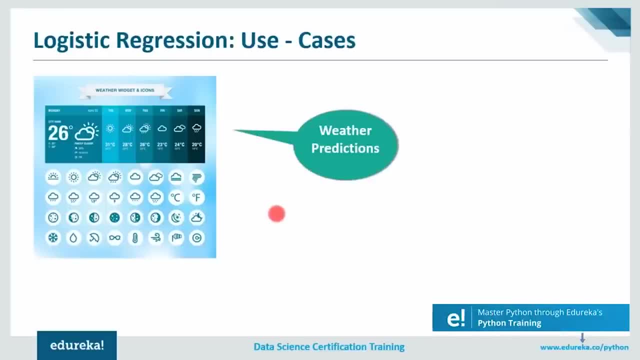 Whereas you need to keep in mind that both linear regression and logistic regression can be used in predicting the weather. So, in that case, linear regression helps you to predict what will be the temperature tomorrow, Whereas logistic regression will only tell you whether it's going to rain or not, or whether it's cloudy or not, which is going to. 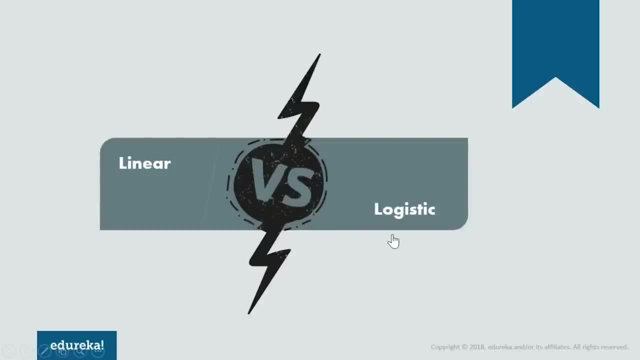 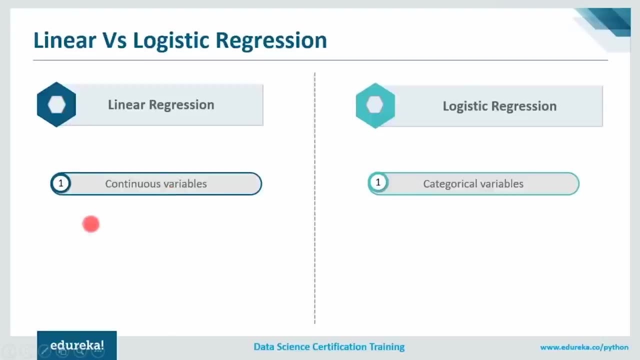 Next, Let us see What are the major differences between linear regression versus logistic regression. Now, first of all, in linear regression we have the value of y as a continuous variable, or the variable which we need to predict a continuous nature, Whereas in logistic regression, 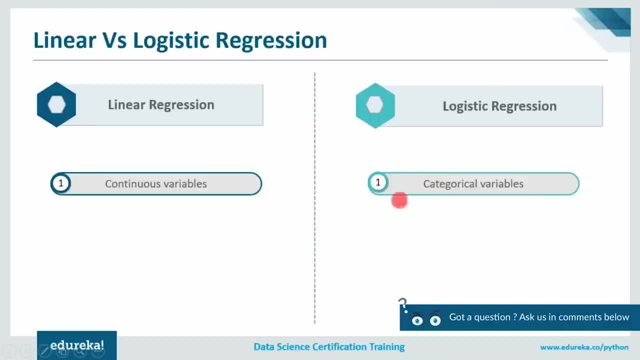 we have the categorical variable. So here the value which you need to predict should be discrete in nature. It should be Either 0 or 1, or it should have just two values to it, For example whether it is raining or it is not raining. 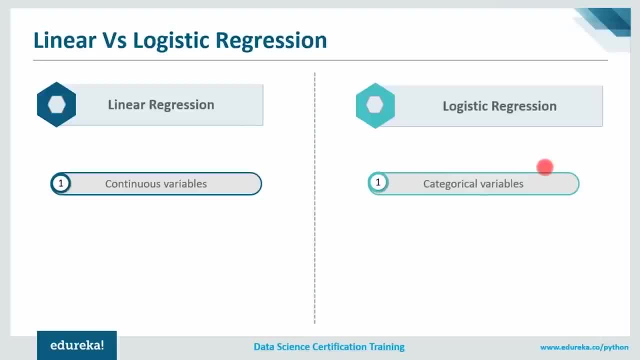 Is it humid outside or it is not humid outside Now? does it going to snow or it is not going to snow? So these are the few example We need to predict where the values are discrete, or you can just predict whether this is happening. 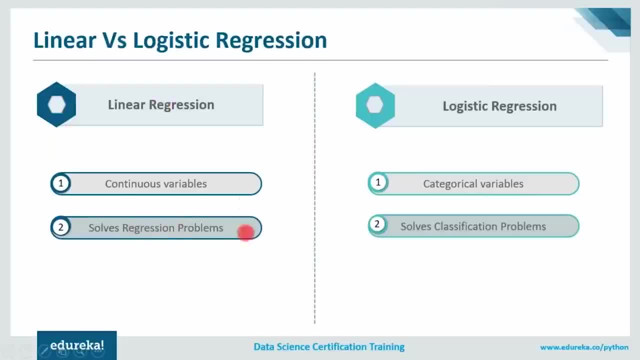 or not. Next, linear regression solves your regression problems. So here you have a concept of independent variable and a dependent variable. So here you can calculate the value of y, which you need to predict using the value of x. So here your y variable, or you can say the value that you need to predict, are in a range. 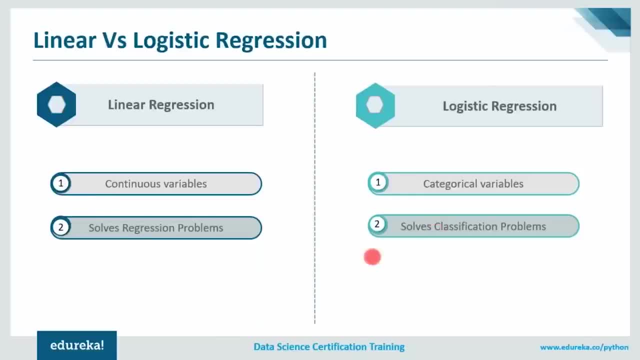 But whereas in logistic regression you have discrete values, So logistic regression basically solves your classification problem. So it can basically classify it and it can just give you result, whether this event is happening or not. So I hope it is pretty much clear till now. 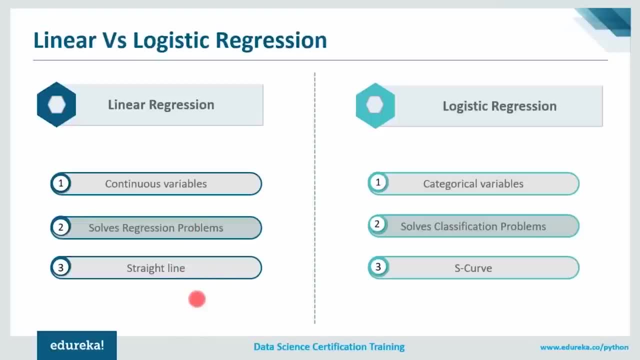 Next, in linear regression, the graph that you have seen is a straight line graph, So over here you can calculate the value of y with respect to the value of x, whereas in logistic regression the curve that we got was a s curve, or you can say the sigmoid curve. 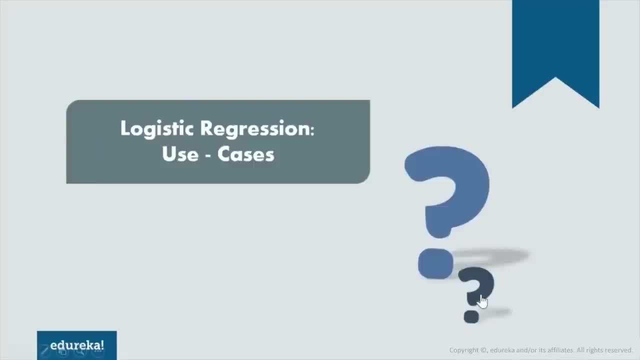 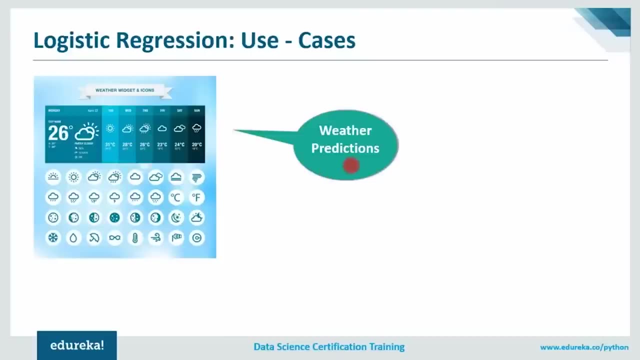 So, using the sigmoid function, you can predict your y values. Moving ahead, let us see the various use cases wherein logistic regression is implemented in real life. So the very first is weather prediction. Now, logistic regression helps you to predict your weather, For example. 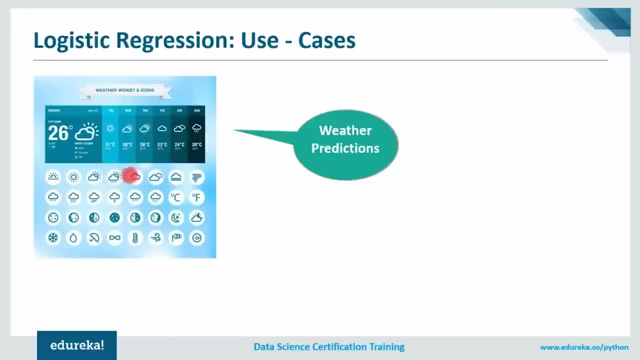 it is used to predict whether it is raining or not, whether it is sunny, is it cloudy or not, So all these things can be predicted using logistic regression, Whereas you need to keep in mind that both linear regression and logistic regression can be used in predicting the weather. 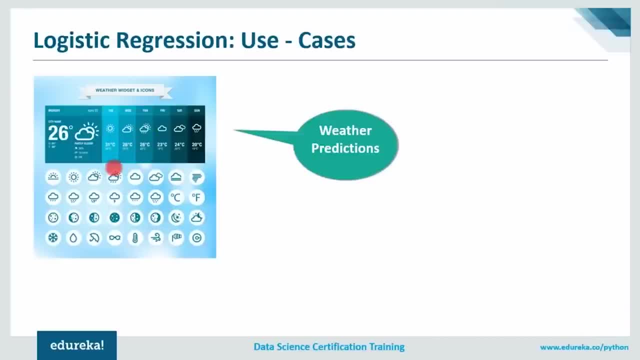 So in that case, linear regression helps you to predict what will be the temperature tomorrow, Whereas logistic regression will only tell you whether it is going to rain or not, or whether it's cloudy or not, which is going to snow or not. So these values are discrete. 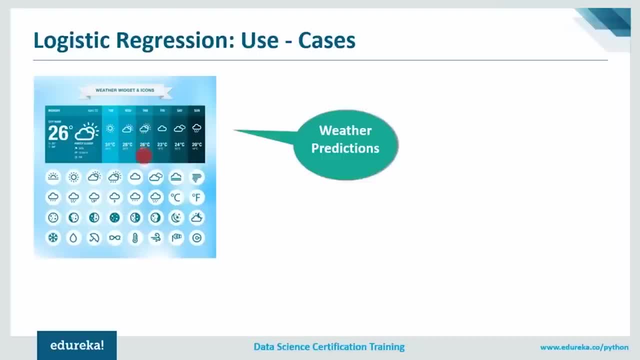 Whereas if you apply linear regression, you will be predicting things like what is the temperature tomorrow or what is the temperature day after tomorrow, and all those things. So these are the slight differences between linear regression and logistic regression. Now moving ahead, we have classification problem. 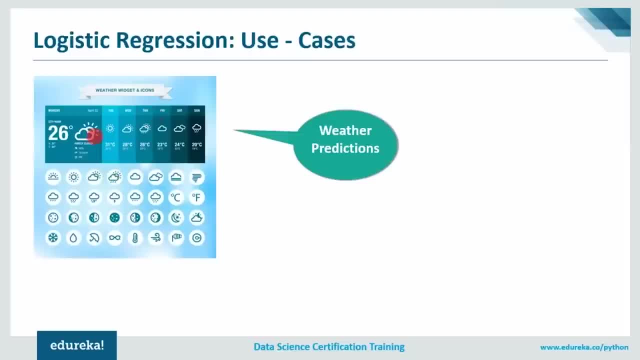 snow or not, So these values are discrete, Whereas if you apply linear regression, you will be predicting things like what is the temperature tomorrow or what is the temperature day after tomorrow and all those things. So these are the slight differences between linear regression and logistic regression. 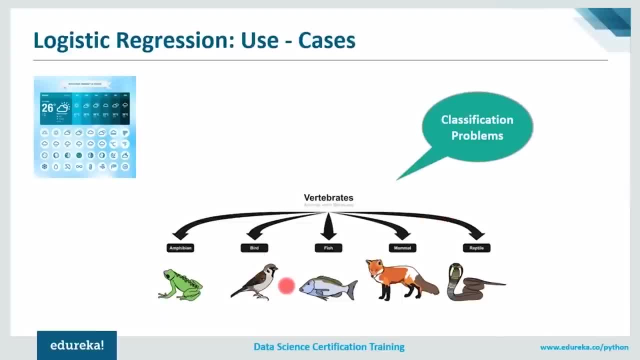 Now moving ahead. we have classification problem. So python performs multi-class classification. So here it can help you tell whether it's a bird or it's not a bird. Then you classify different classifications, Let's say whether it's a dog or it's not a dog. 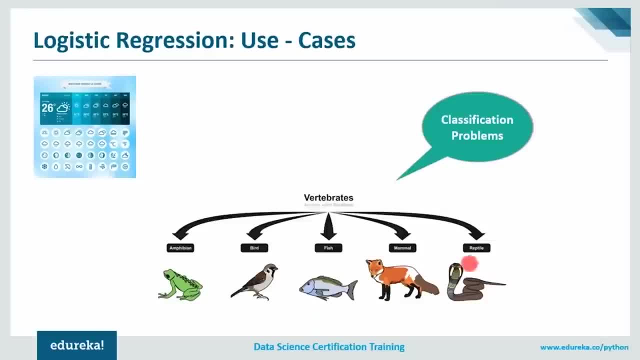 Similarly, you can check it for reptile, whether it's a reptile or not a reptile. So in logistic regression it can perform multi-class classification. So this point I have already discussed, that it is used in classification problems. Next, it also helps you to determine the illness as well. 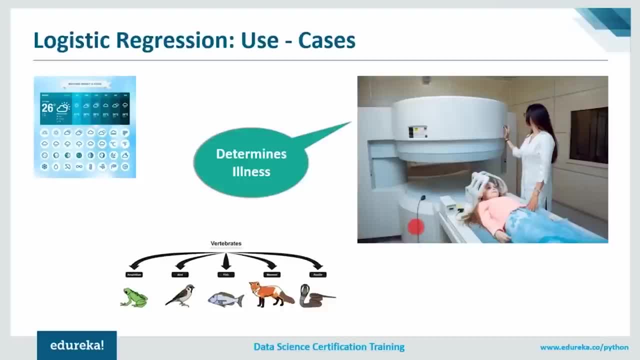 So let me take an example. Let's say a patient goes for routine checkup in hospital. So what doctor will do? it will perform various tests on the patient and will check whether the patient is actually ill or not. So what will be the feature? 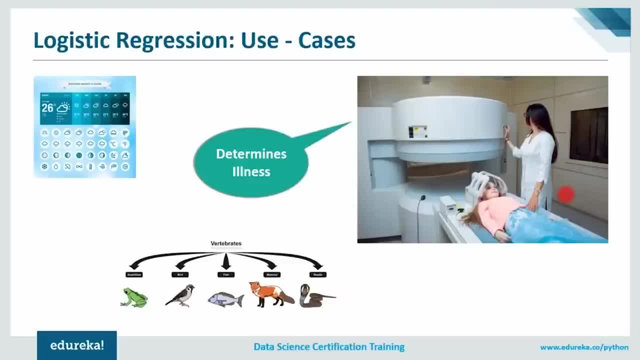 So doctor can check the sugar level, the blood pressure. then what is the age of the patient? is it very small or is it an old person? then what is the previous medical history of that patient? and all of these features will be recorded by the doctor. and finally, doctor checks the patient data and determines the outcome. 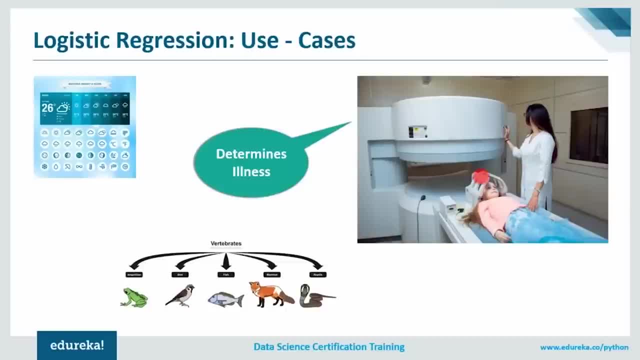 of an illness and the severity of illness. So using all the data, a doctor can identify whether a patient is ill or not. So these are the various use cases in which you can use logistic regression. Now, I guess, enough of theory, But so let's move ahead and see some of the practical implementation. 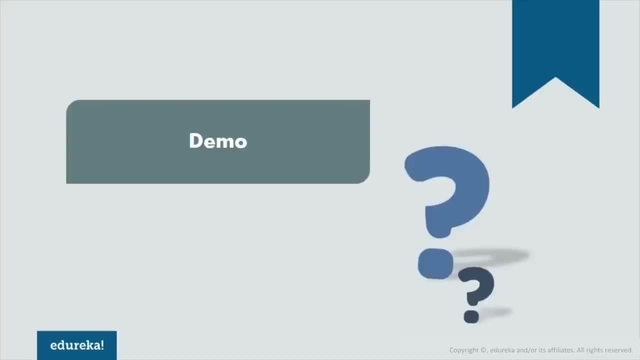 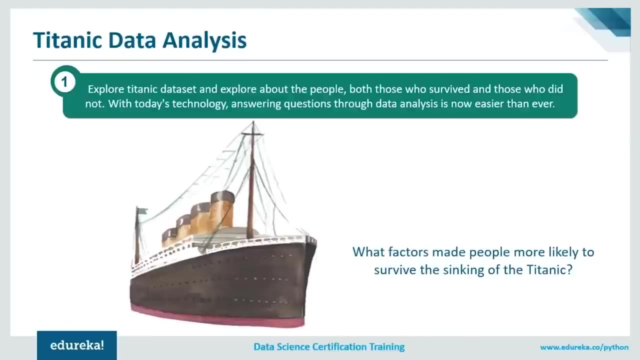 of logistic regression. So over here I'll be implementing two projects wherein I have the data set of a Titanic. over here will predict what factors made people more likely to survive the sinking of the Titanic ship and in my second project will see the data analysis on the SUV. 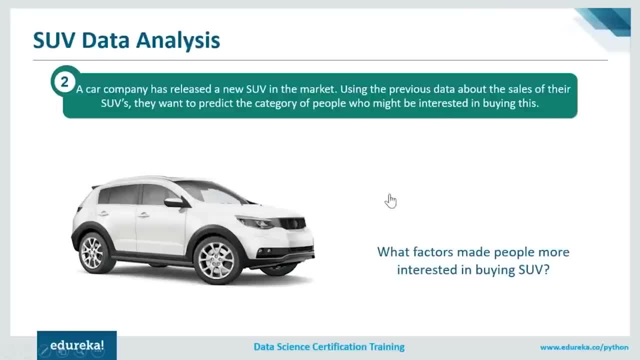 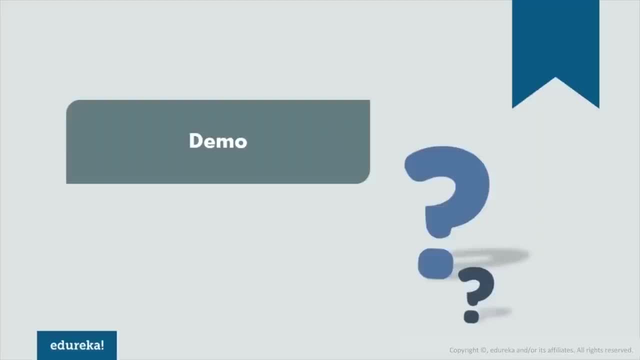 cars. So over here we have the data of the SUV cars, who can purchase it and what factors made people more interested in buying SUV. So these will be the major questions as to why you should implement logistic regression and what output will you get by it. 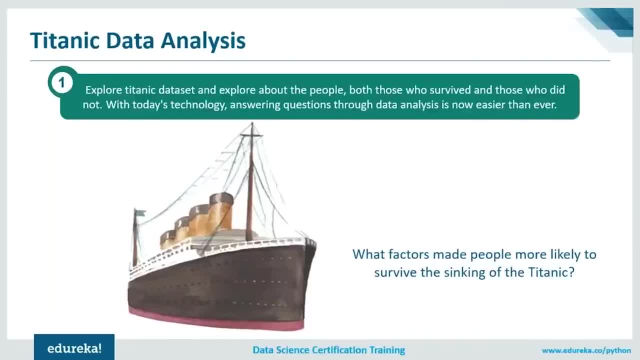 So let's start by the very first project, that is, Titanic data analysis. So some of you might know that there was a ship called as Titanic, which basically hit an iceberg and it sunk to the bottom of the ocean and it was a big disaster at that time because it was the 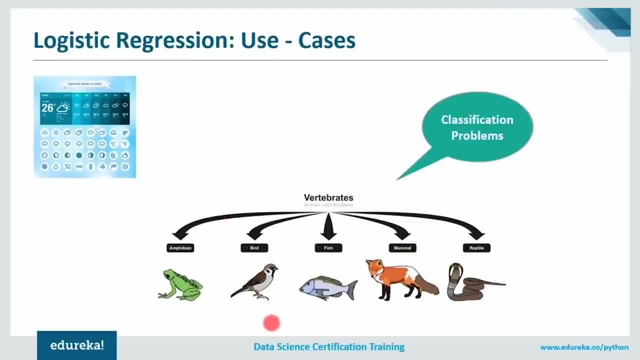 So Python performs multi-class classification. So here it can help you tell whether it's a bird or it's not a bird. Then you classify different kind of mammals, Let's say whether it's a dog or it's not a dog. Similarly, 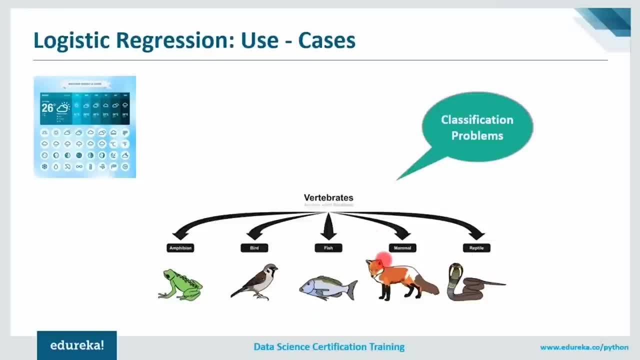 you can check it for reptile, whether it's a reptile or not a reptile. So in logistic regression it can perform multi-class classification. So this point I have already discussed that it is used in classification problems. Next, it also helps you to determine the illness as well. 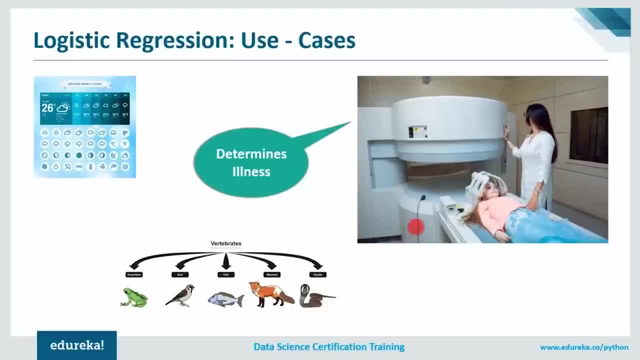 So let me take an example. Let's say a patient goes for routine checkup in hospital. So what doctor will do is it will perform various tests on the patient and will check whether the patient is actually ill or not. So what will be the features? 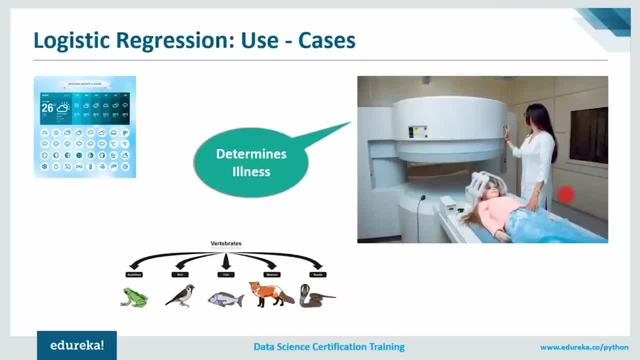 So doctor can check the sugar level, the blood pressure. Then what is the age of the patient? Is it very small or is it an old person? Then what is the previous medical history of that patient? And all of these features will be recorded by the doctor. 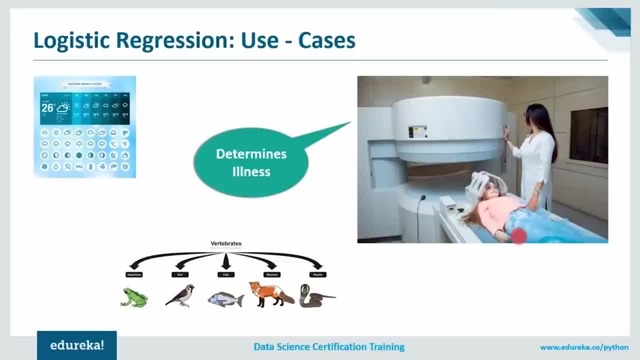 And finally, doctor checks the patient data and determines the outcome of an illness and the severity of illness. So, using all the data, a doctor can identify whether a patient is ill or not. So these are the various use cases in which you can use logistic regression. 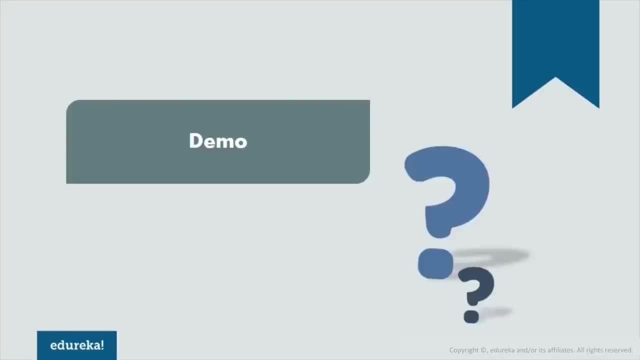 Now, I guess, enough of theory part, So let's move ahead and see some of the practical implementation of logistic regression. So over here I'll be implementing two projects wherein I have the data set of a Titanic. So over here we'll predict what factors made people more likely to survive the sinking of. 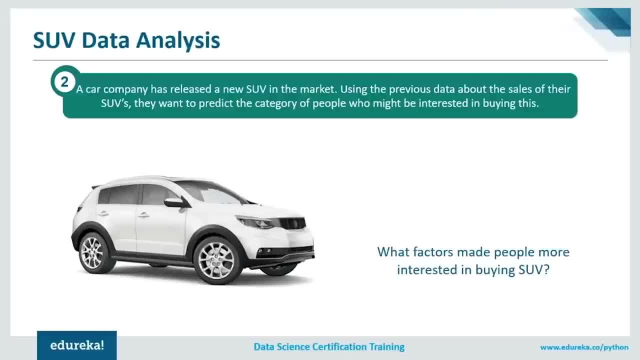 the Titanic ship, And in my second project we'll see the data analysis on the SUV cars. So over here we have the data of the SUV cars, who can purchase it and what factors made people more interested in buying SUV. So these will be the major questions as to why you should implement logistic. 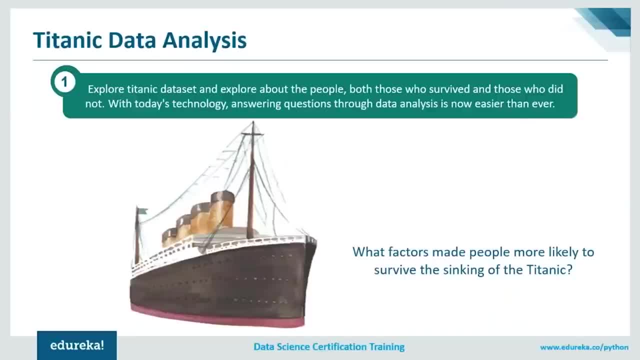 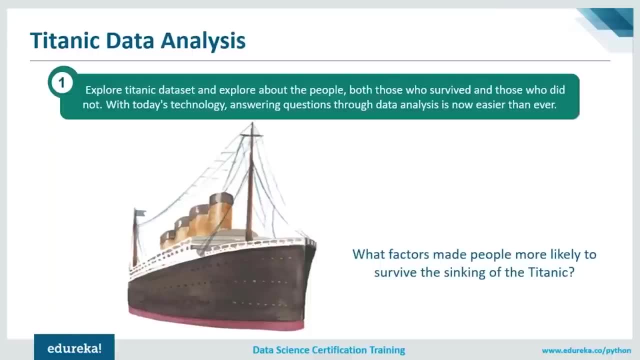 regression, and what output will you get by it? So let's start by the very first project, that is, Titanic data analysis. So some of you might know that there was a ship called as Titanic, which basically hit an iceberg and it sunk to the bottom of the ocean. 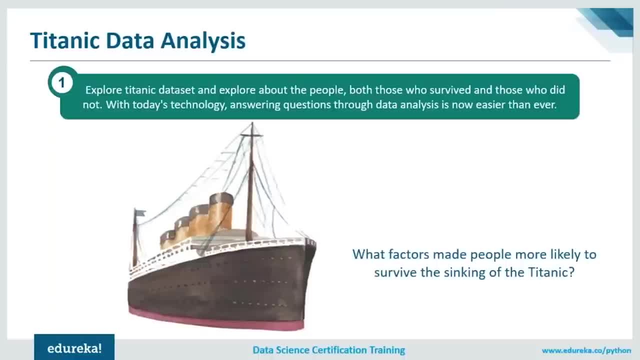 And it was a big disaster at that time because it was the first voyage of the ship and it was supposed to be really, really strongly built and one of the best ships of that time. So it was a big disaster of that time And, of course, 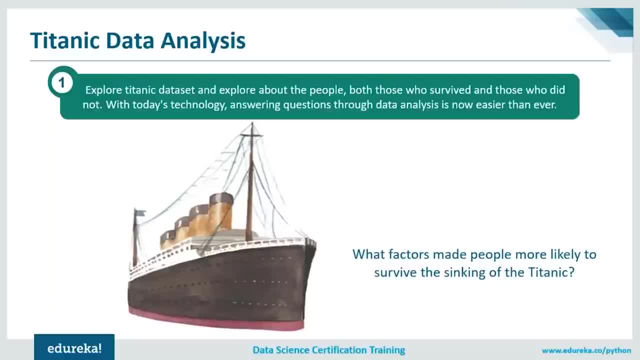 there's a movie about this as well, So many of you might have watched it. So what we have? we have data of the passengers- those who survived and those who did not survive in this particular tragedy. So what you have to do, you have to look at this data and analyze which. 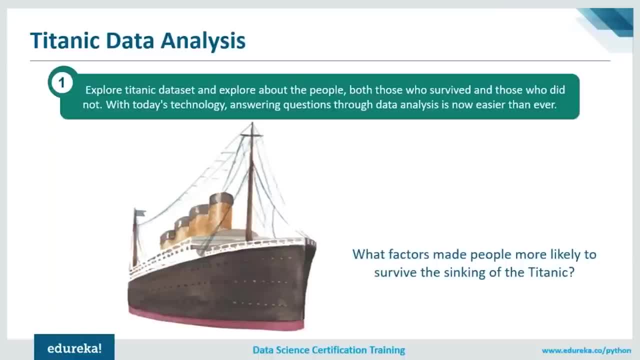 first voyage of the ship and it was supposed to be really, really strongly built and one of the best ships of that time. So it was a big disaster of that time And, of course, there's a movie about this as well, So many of you might have watched it. 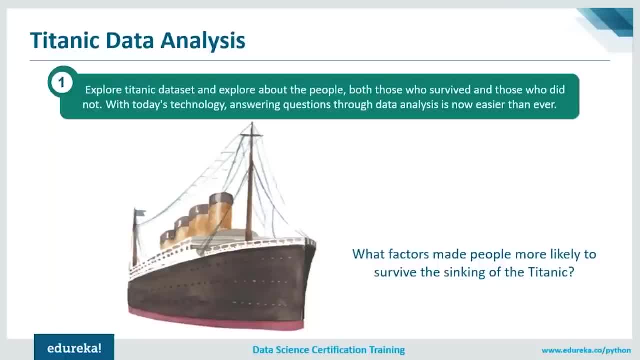 So what we have? we have data of the pattern Passengers, those who survived and those who did not survive in this particular tragedy. So what you have to do, you have to look at this data and analyze which factors would have been contributed the most to the chances. 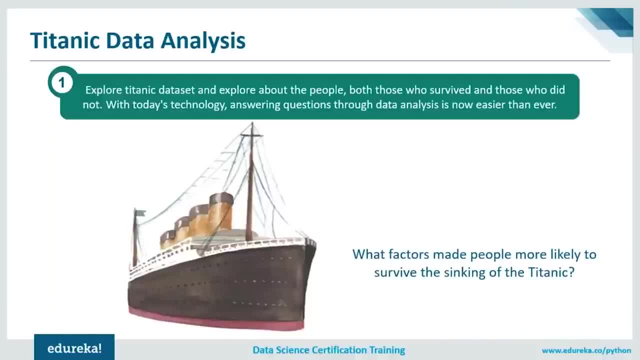 of a person- survival on the ship or not. So using the logistic regression, we can predict whether the person survived or the person died. now, apart from this will also have a look with the various features along with that. So first let us explore the data set. 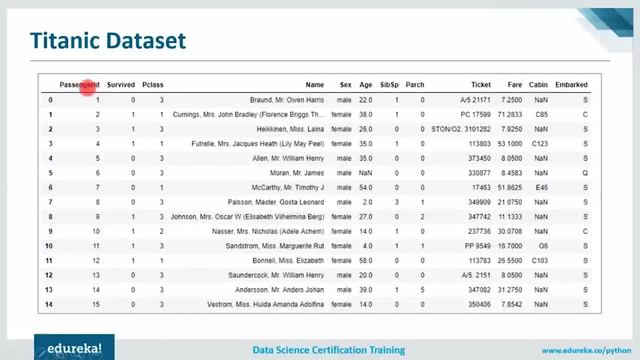 So over here we have the index value, Then the first column is passenger ID, then my next column is survived. So over here we have two values, a zero and a one. so zero stands for did not survive and one stands for survive. So this column is categorical, where the values are discrete. next, 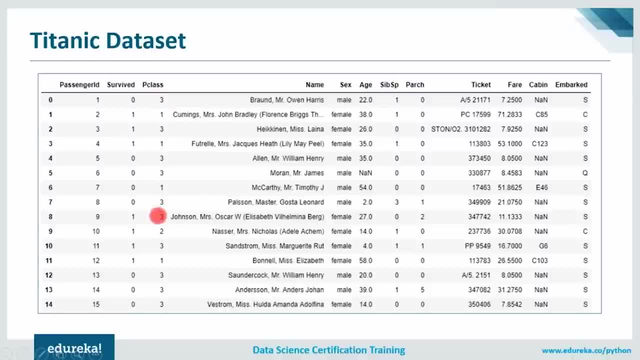 We have passenger class over here. We have three values: one, two and three. So this basically tells you that whether a passenger is traveling in the first class, second class or third class, then we have the name of the passenger, We have the sex or you can say the gender of the passenger. whether 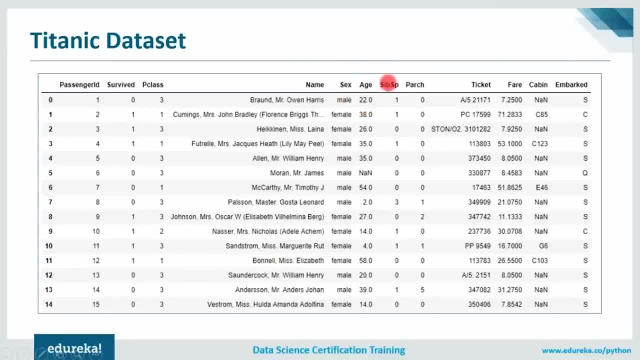 passenger is a male or female. then we have the age, we have the, So this basically means the number of siblings or the spouses aboard the Titanic. So over here we have values such as one, zero and so on. then we have patch. So patch is basically the number of parents or children aboard the. 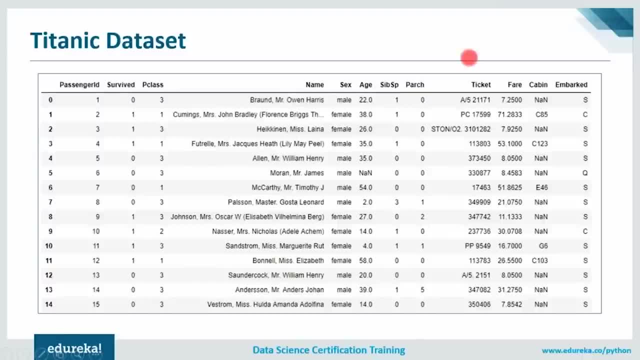 Titanic over here. We also have some values. then we have the ticket number, We have the fare, We have the cabin number and we have the embarked column. So in my embarked column we have three values. We have S, C and Q. 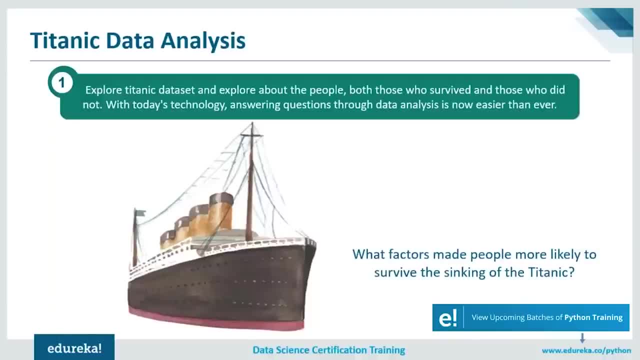 factors would have been contributed the most to the chances of a person's survival on the ship or not. So, using the logistic regression, we can predict whether the person survived or the person died. Now, apart from this, we also have a look with the various features along with that. 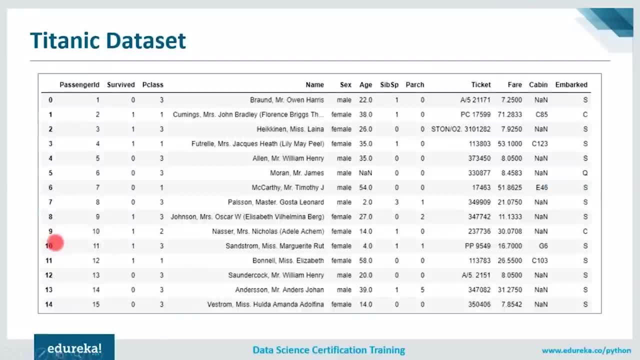 So first let us explore the data set. So over here we have the index value, Then the first column is passenger ID, Then my next column is survived. So over here we have two values, a zero and a one. So zero stands for did not survive and one stands for survive. 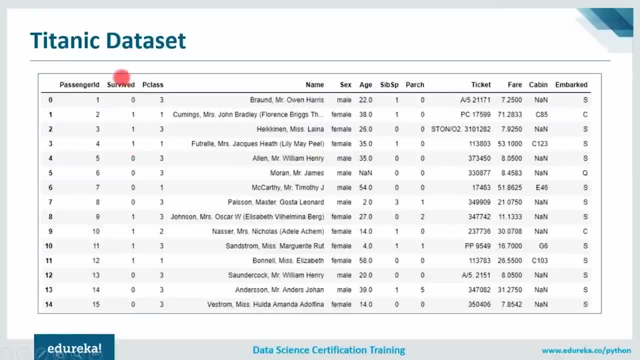 So this column is categorical, where the values are discrete. Next, we have passenger class. So over here we have three values: one, two and three. So this basically tells you that whether a passenger is traveling in the first class, second class or third class, 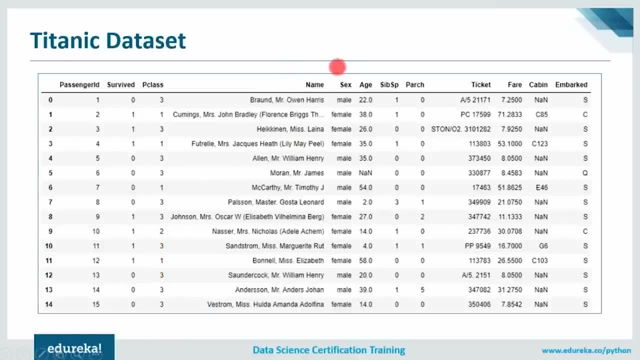 Then we have the name of the passenger, We have the sex, or you can say the gender of the passenger, whether passenger is a male or female. Then we have the age. We have the Sib, SP. So this basically means the number of siblings or the spouses aboard the 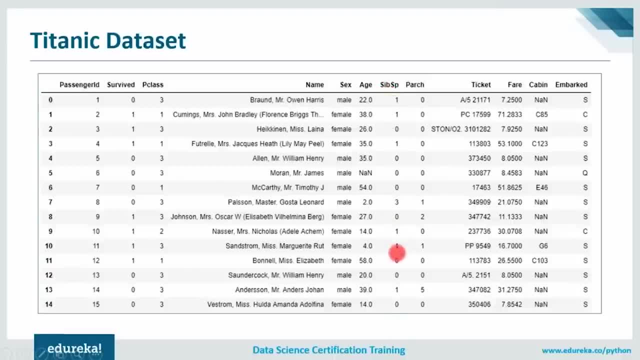 Titanic. So over here we have values such as one zero and so on. Then we have patch. So patch is basically the number of parents or children aboard the Titanic. So over here we also have some values. Then we have the ticket number. 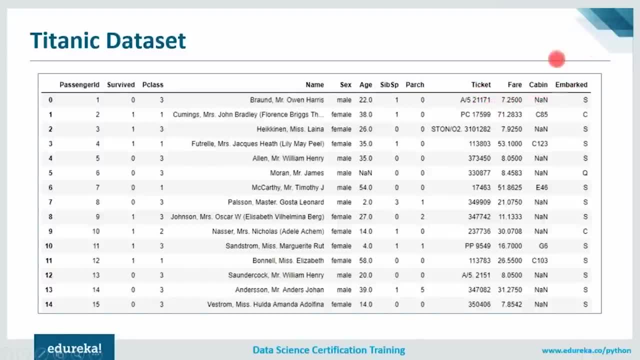 We have the fare, We have the cabin Number and we have the embarked column. So in my embarked column we have three values. We have S, C and Q. So S basically stands for Southampton, C stands for Cherbourg and Q stands for Kuenstown. 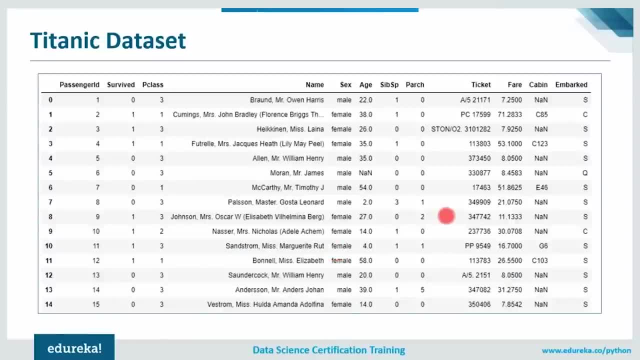 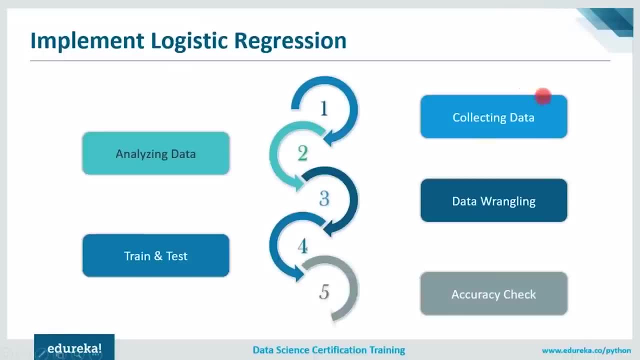 So these are the features that we'll be applying our model on. So here we will perform various steps, and then we'll be implementing logistic regression. So now these are the various steps which are required to implement any algorithm. So now, in our case, 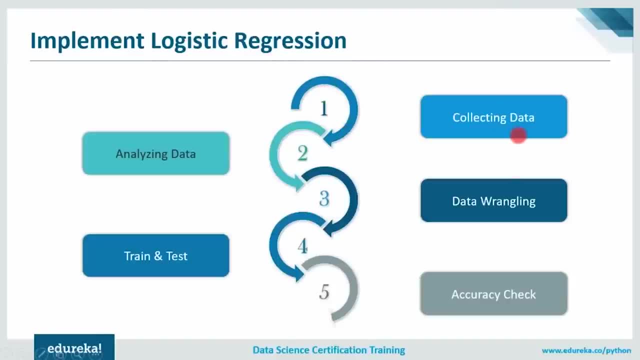 we are implementing logistic regression. So very first step is to collect your data or to import the library that I used for collecting your data and then taking it forward. Then my second step is to analyze your data. So over here I can go through the various fields and then I can analyze the data. 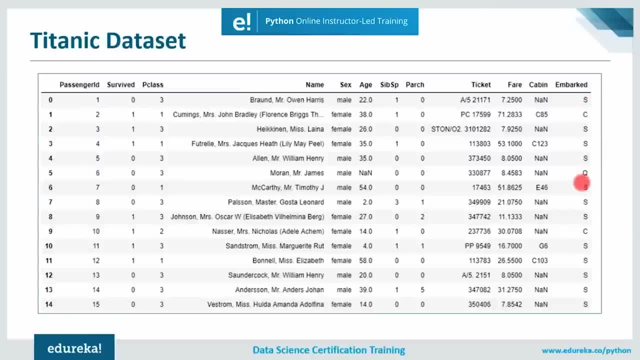 So S basically stands for Southampton, C stands for Cherbourg and Q stands for Kuenstown. So these are the features that we'll be applying our model on. So here we will perform various steps and then we'll be implementing logistic regression. So now these are the various steps which are required to implement. 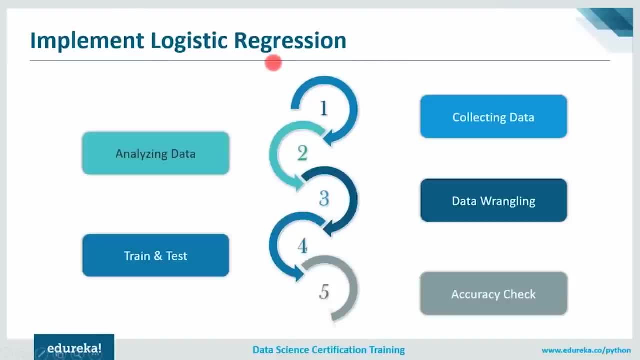 any algorithm. So now, in our case, we are implementing logistic regression. So very first step is to collect your data, or to import the libraries that are used for collecting your data and then taking it forward. Then my second step is to analyze your data. 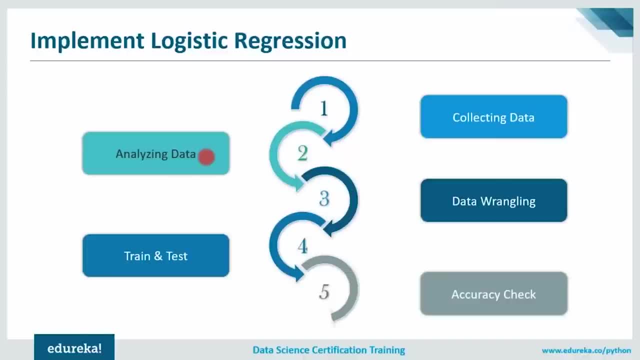 So over here I can go through the various fields And then I can analyze the data. I can check: did the females or children survive better than the males? or did the rich passenger survive more than the poor passenger? or did the money matter, as in who paid more to get into the ship? 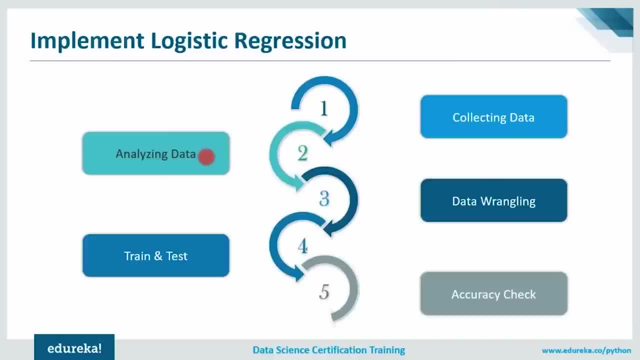 what they evacuated first. and what about the workers? does the worker survived, or what is the survival rate if you were the worker in the ship and not just a traveling passenger? So all of these are very, very interesting questions and you would be going through all of them one by one. 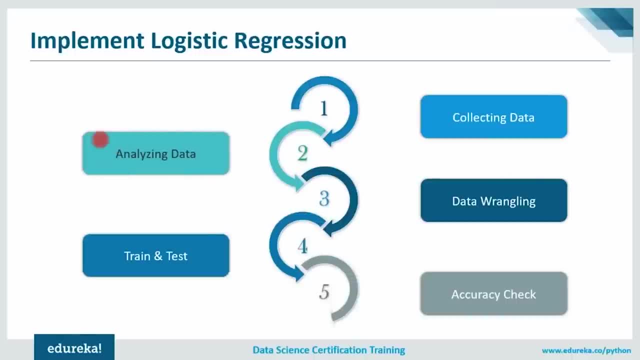 So in this stage, you need to analyze your data and explore your data As much as you can. then my third step is to wrangle your data now. data wrangling basically means cleaning your data. So over here you can simply remove the unnecessary items or, if you, 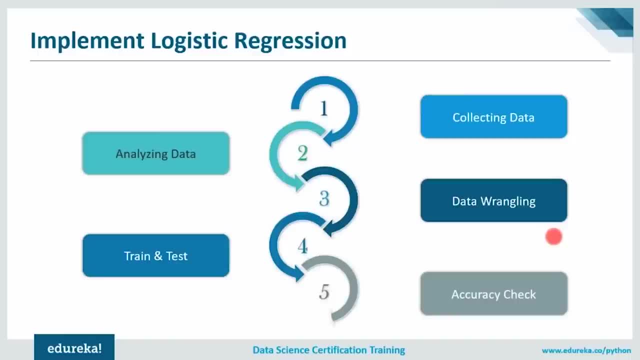 have a null values in the data set, you can just clear that data and then you can take it forward. So in this step you can build your model using the train data set and then you can test it using a test over here. You will be performing a split which basically split your data set. 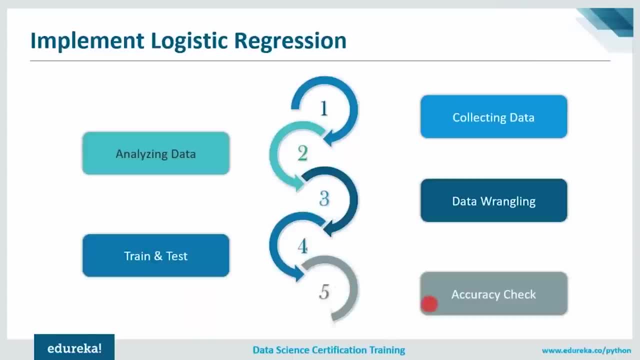 into training and testing data set and finally, you will check the accuracy So as to ensure how much accuracy Your values are. so I hope you guys got these five steps that you're going to implement in logistic regression. So now let's go into all these steps in detail. 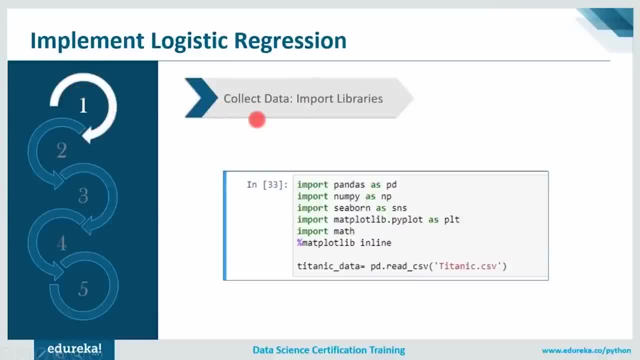 So, number one, we have to collect your data, or you can say, import the libraries So it may show you the implementation part as well. So I just open my Jupiter notebook and I just implement all of these steps side by side. So, guys, this is my Jupiter notebook. 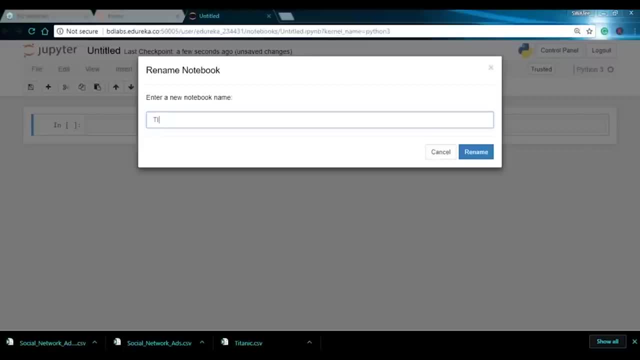 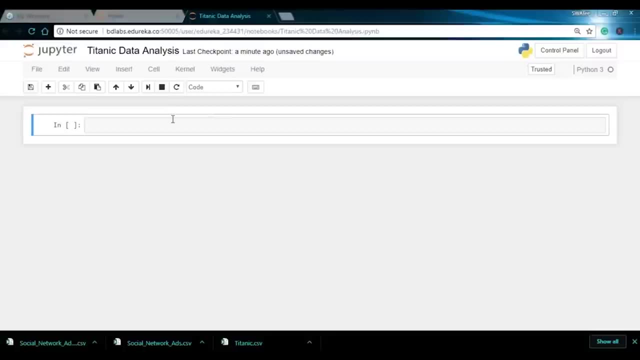 So first let me just rename Jupiter notebook to, let's say, Titanic data analysis. Now our first step was to import all the libraries and collect the data, So let me just import all the libraries first. So first of all I'll import pandas. 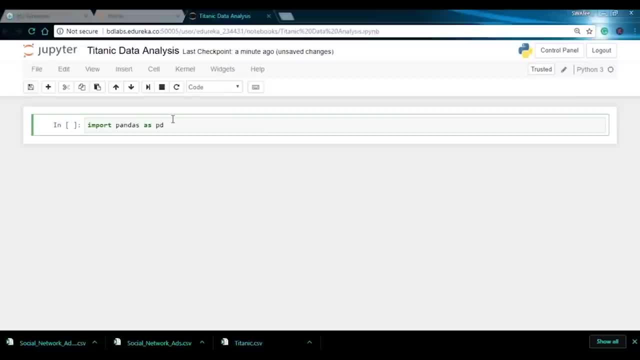 So pandas is used for data analysis. So I'll say: import pandas as PD. then I'll be importing numpy, So I'll say: import numpy as NP. So numpy is a library in Python which basically stands for numerical Python and it is widely used to perform any scientific computation. 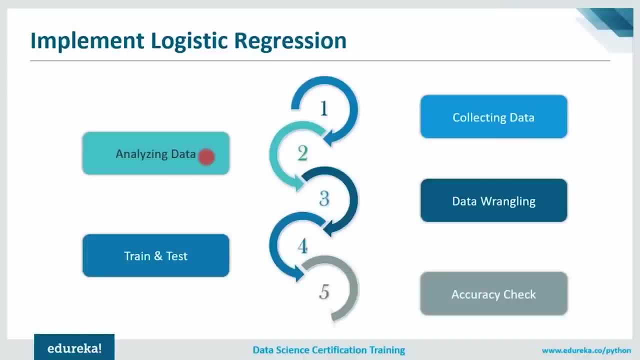 I can check. did the females or children survive better than the males? or did the rich passenger survive more than the poor passenger? or did the money matter, as in who paid more to get into the ship, what they evacuated first? and what about the workers? does the worker survived or what is the 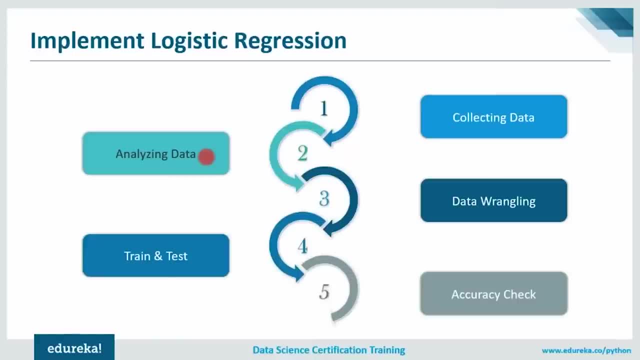 survival rate if you were the worker in the ship and not just a traveling passenger? So all of these are very, very interesting questions and you would be going through all of them one by one. So in this stage, you need to analyze your data and explore your data as much as you can. 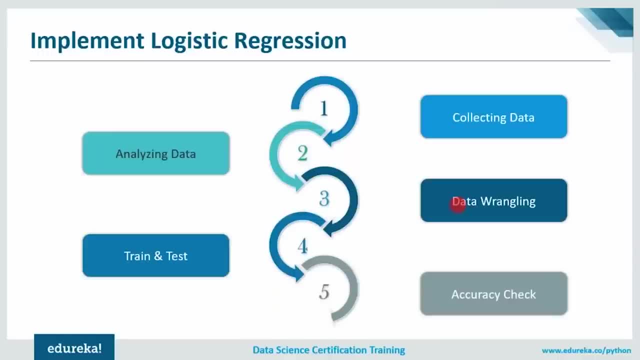 Then my third step is to wrangle your data. Now, data wrangling basically means cleaning your data. So over here you can simply remove the unnecessary items, or, if you have a null values in the data set, you can just clear that data and then you can take it forward. 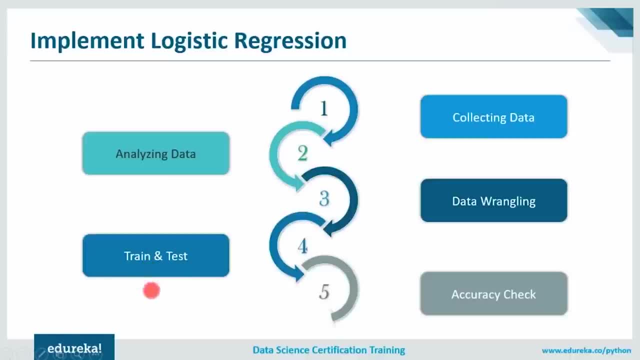 So in this step you can build your model using the train data set and then you can test it using a test. over here We will be performing the split, which basically split your data set into training and testing data set, and finally you will check the accuracy. 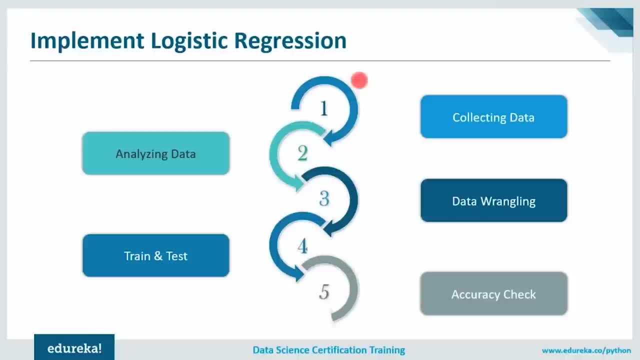 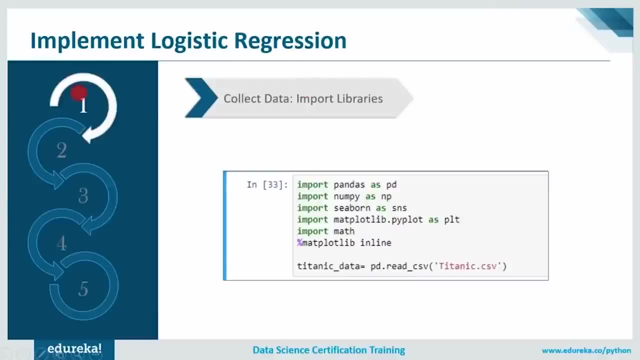 So as to ensure how much accurate your values are. So I hope you guys got these five steps that we're going to implement in logistic regression. So now let's go into all these steps in detail. So, number one: we have to collect your data, or you can say: import the libraries. 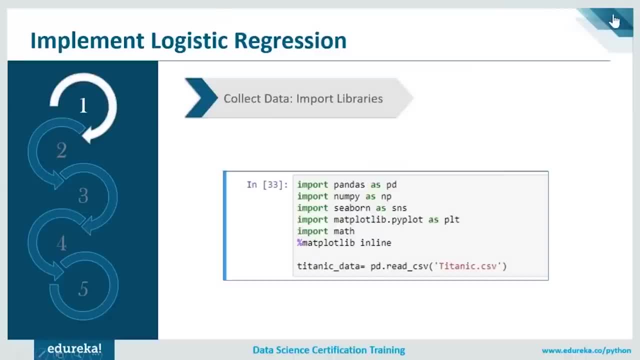 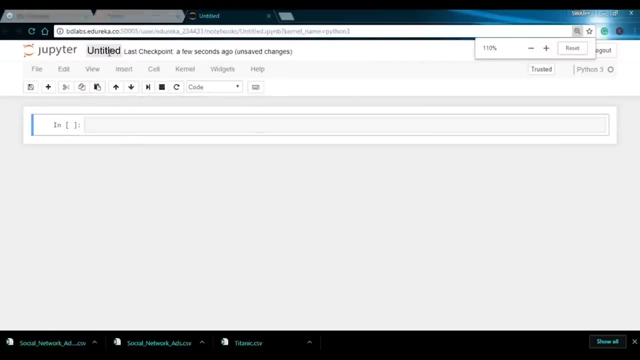 So it may show you the implementation part as well. So I just open my Jupiter notebook and I just implement all of these steps side by side. So, guys, this is my Jupiter notebook. So first let me just rename Jupiter notebook to, let's say, Titanic data analysis. 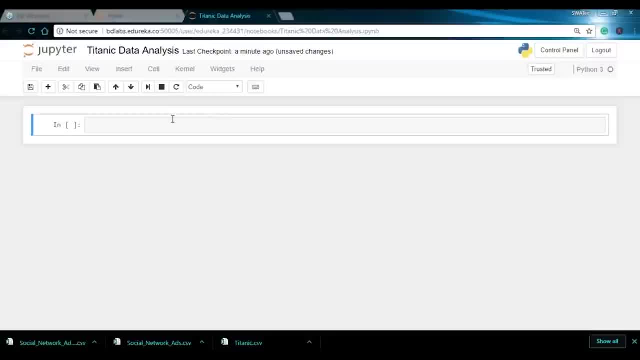 Now our first step was to import all the libraries and collect the data. So let me just import all the libraries first. So first of all I'll import pandas. So pandas is used for data analysis. So I'll say: import pandas as PD, then I'll be importing numpy. 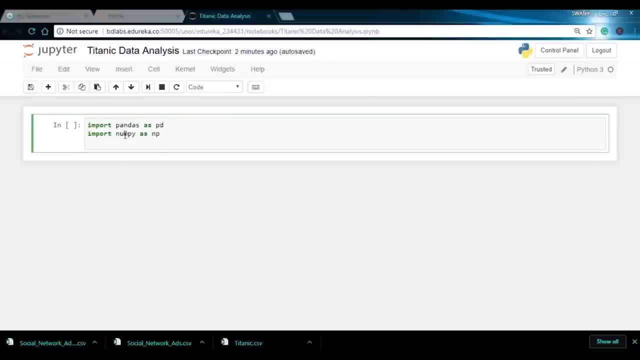 So I'll say: import numpy as NP, So numpy is a library In Python which basically stands for numerical Python, and it is widely used to perform any scientific computation. Next we'll be importing seaborn, So seaborn is a library for statistical plotting. 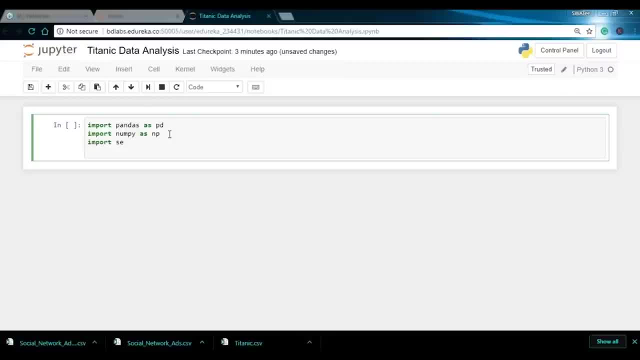 Next we'll be importing seaborn, So seaborn is a library for statistical plotting. So I'll say: import seaborn as SNS. I'll also import matplotlib, So matplotlib library is again for plotting. So I'll say: import matplotlib dot pyplot as PLD. 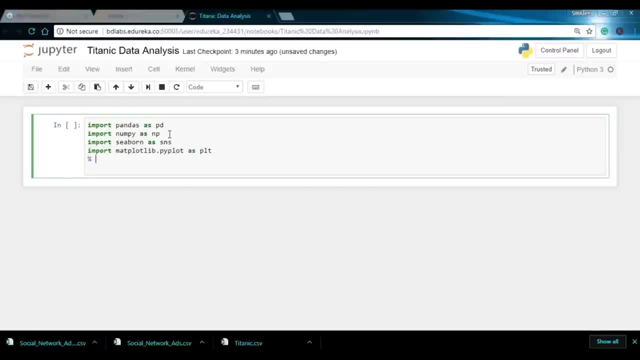 Now to run this library in Jupiter notebook, All I have to write in is percentage matplotlib inline. Next, I'll be importing one module as well So as to calculate the basic mathematical functions. so I'll say: import maths. So these are the libraries that I'll be needing in this Titanic. 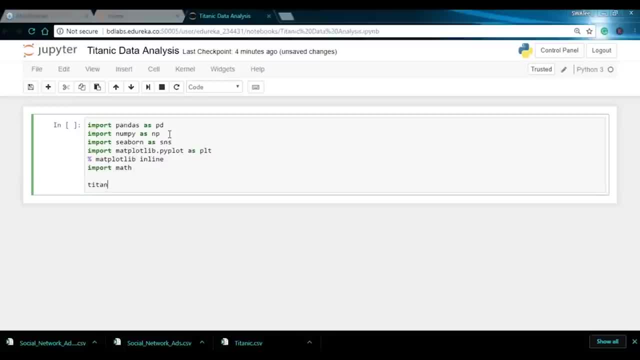 data analysis. So now let me just import my data set. So I'll take a variable, Let's say Titanic data, and using the pandas I will just read my CSV, or you can say the data set. I'll write the name of my data set, that is, Titanic dot CSV. 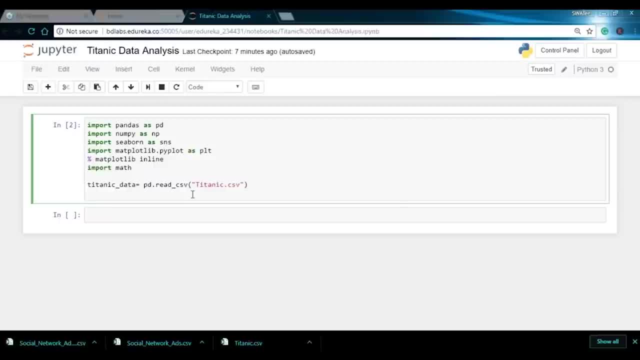 Now I have already showed you the data set, So over here let me just print the top 10 rows. So for that I'll just say: I'll take the variable Titanic data dot head and I'll say the top 10 rows. 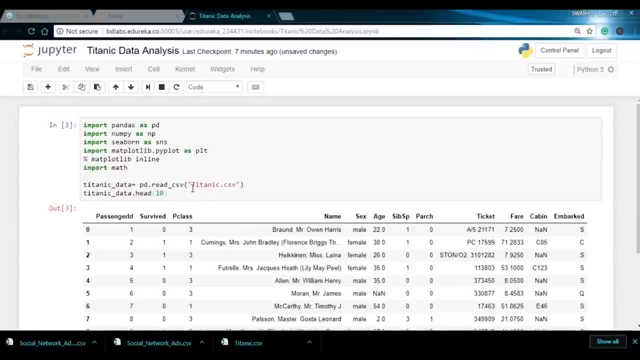 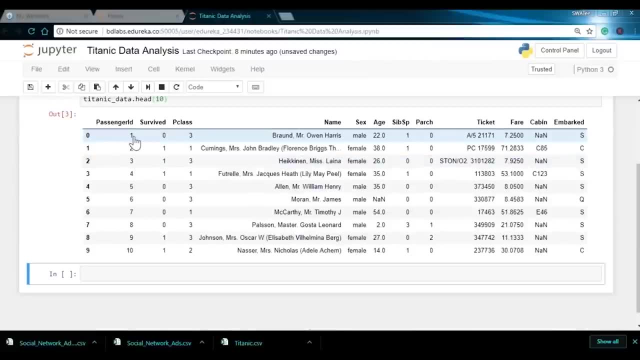 So now I'll just run this. so to run this, So I just have to press shift plus enter, or else you can just directly click on the cell. So over here I have the index, We have the passenger ID, which is nothing but again the index. 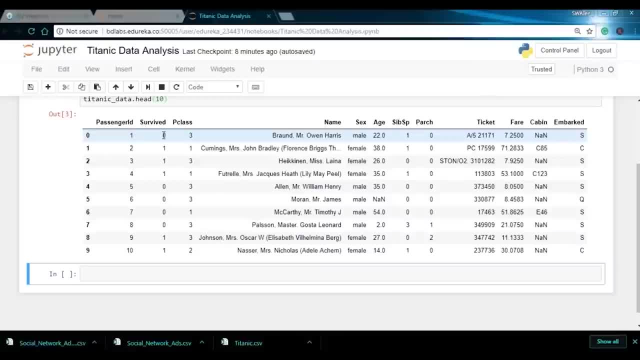 which is starting from 1. then we have the survive column, which has the categorical values, or you can say the discrete values, which is in the form of 0 or 1. then we have the passenger class. We have the name of the passenger, sex, age and so on. 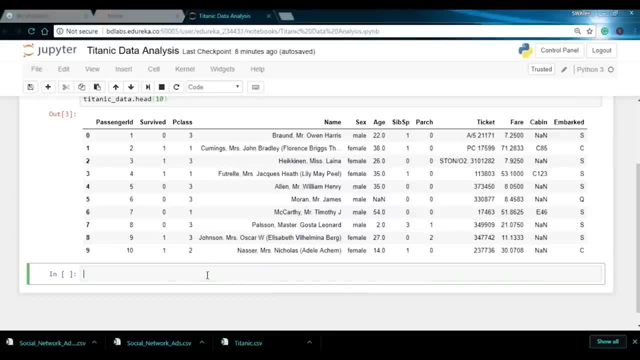 So this is the data set that I'll be going forward with next latest print: the number of passengers which are there in this original data set. for that I just simply type in print, I'll say number of passengers And using the length function. 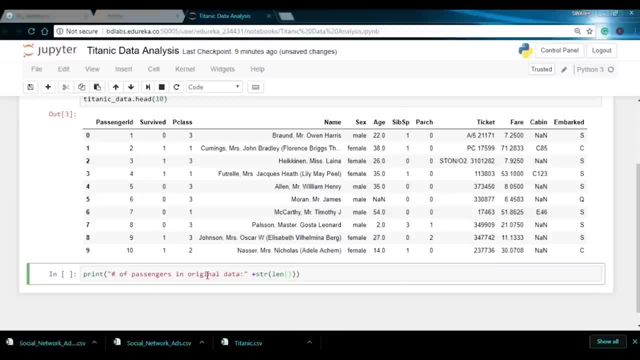 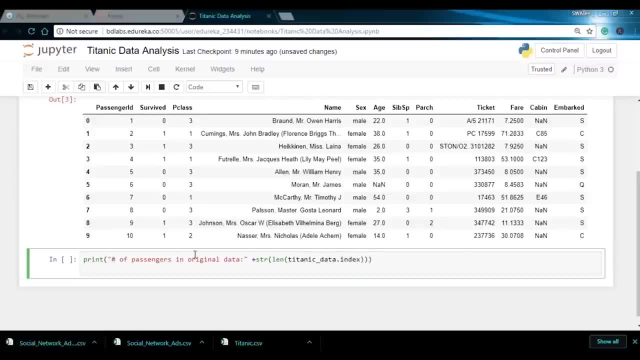 I can calculate the total length. So I'll say length and inside this I'll be passing this variable which is Titanic data. So I'll just copy it from here. I just paste it: dot index and next. so let me just print this one. 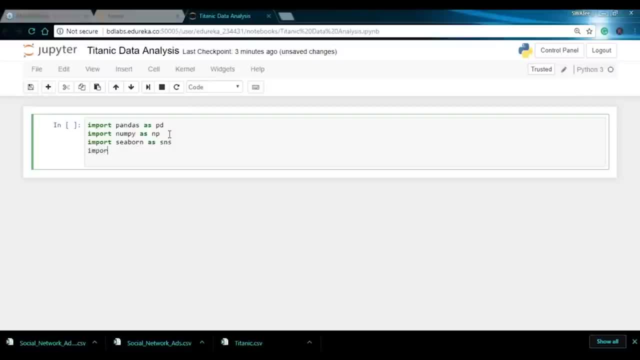 So I'll say: import seaborn as SNS. I'll also import matplotlib. So matplotlib library is again for plotting. So I'll say: import matplotlib dot pyplot as PLD. Now to run this library. in Jupiter notebook All I have to write in is percentage matplotlib inline. 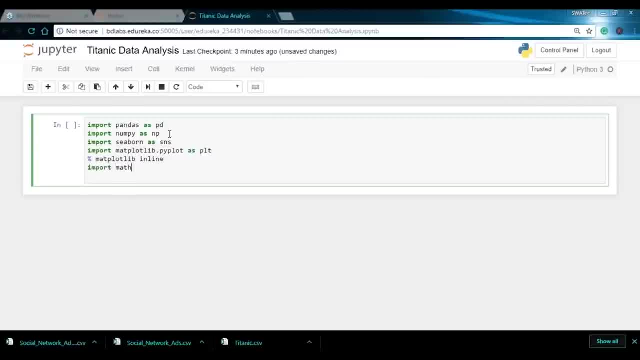 Next, I'll be importing one module as well, So as to calculate the basic mathematical functions. so I'll say: import maths. So these are the libraries that I'll be needing in this Titanic data analysis. So now let me just import my data set. 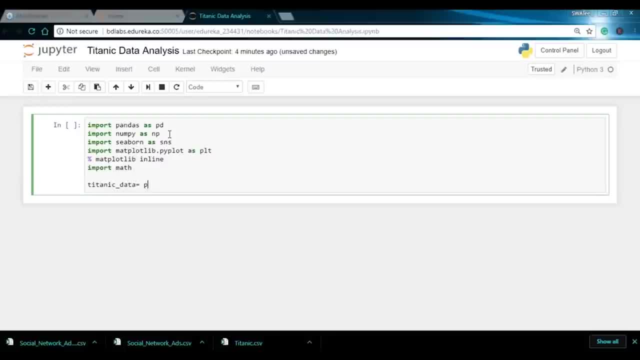 So I'll take a variable, Let's say Titanic data, and using the pandas, I will just read my CSV, or you can say the data set. I'll write the name of my data set, that is, Titanic dot CSV. Now I have already showed you the data set. 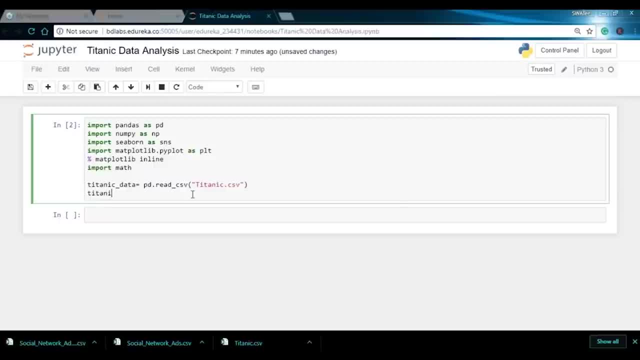 So over here let me just print the top 10 rows. So for that I'll just say: I'll take the variable Titanic data dot head and I'll say the top 10 rows. So now I'll just run this. so to run this, 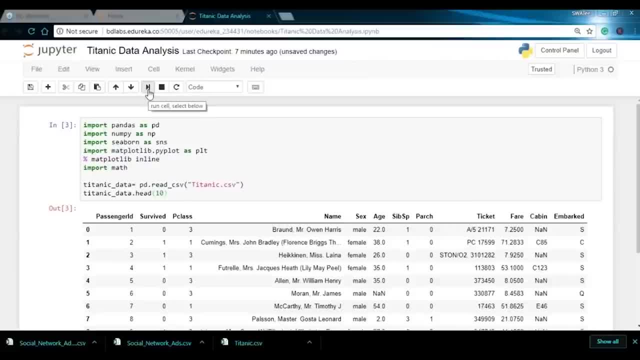 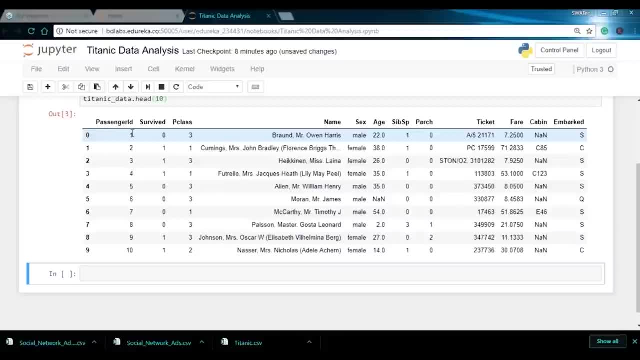 So I just have to press shift plus enter, or else You can just directly click on the cell. So over here I have the index, We have the passenger ID, which is nothing but again the index which is starting from one. then we have the survive column. 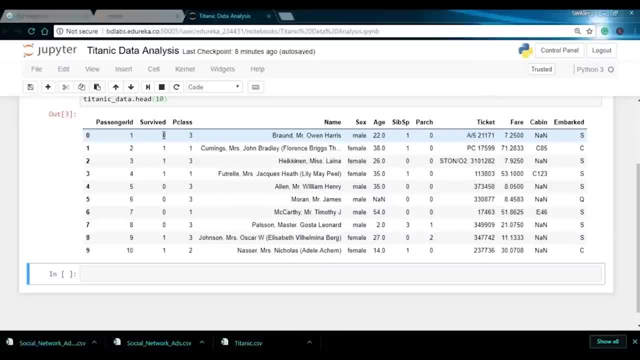 which has the categorical values, or you can say the discrete values, which is in the form of 0 or 1. then we have the passenger class, We have the name of the passenger, sex, age and so on. So this is the data set that I'll be going forward with next. 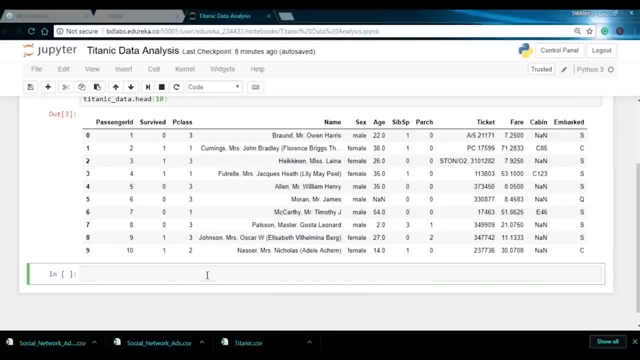 Let us print the number of passengers which are there in this original data set. for that I'll just simply type in print. I'll say number of passengers And using the length function I can calculate the total length. So I'll say length and inside this I'll be passing this variable. 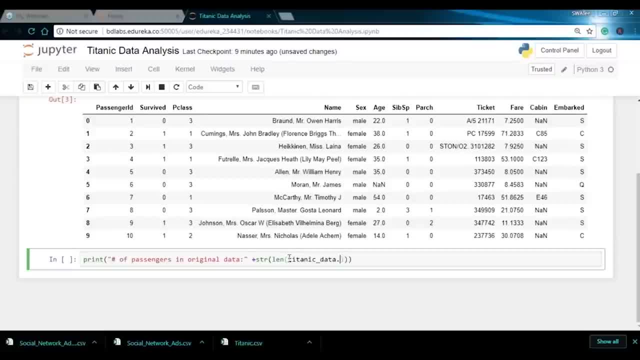 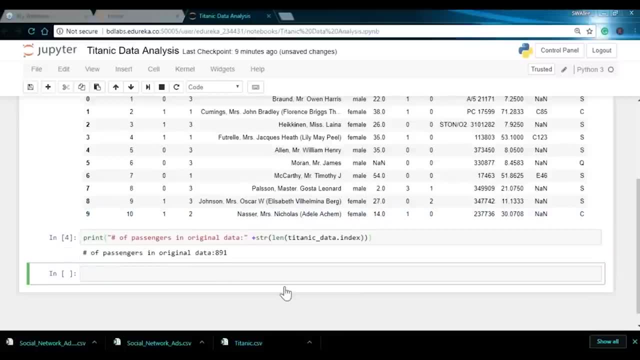 which is Titanic data, So I'll just copy it from here. I just paste it: dot index and next. so let me just print this one. So here the number of passengers which are there in the original data set we have is 891, so around this number were traveling. 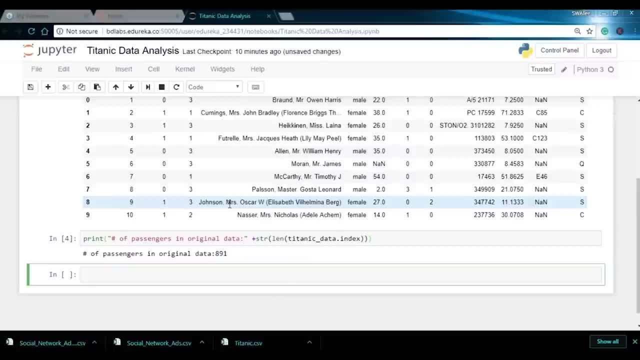 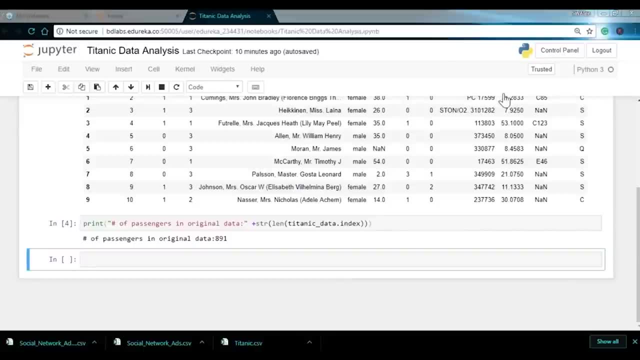 in the Titanic ship. So over here, My first step is done, where you have just collected data, imported all the libraries and find out the total number of passengers which are traveling in Titanic. So now let me just go back to presentation and let's see. 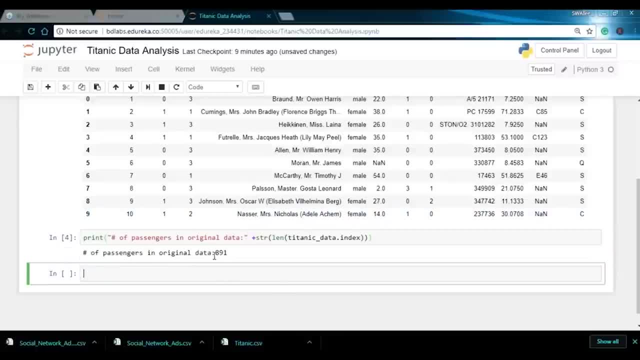 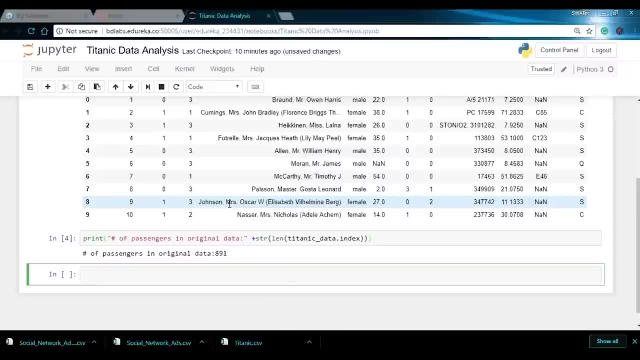 So here, the number of passengers which are there in the original data set we have is 891.. So around this number were traveling in the Titanic ship. So over here, My first step is done. So you have just collected data, imported all the libraries. 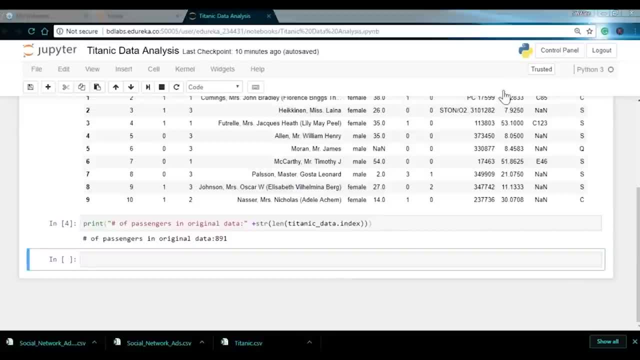 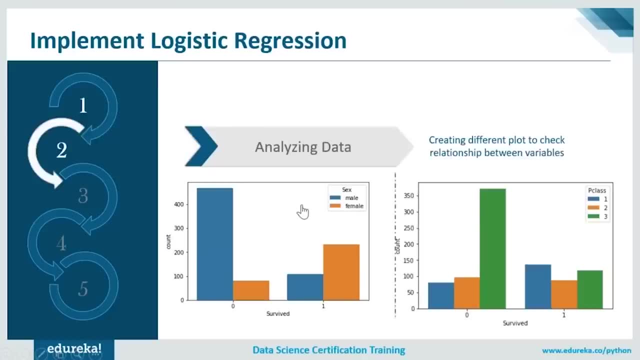 and find out the total number of passengers which are traveling in Titanic. So now let me just go back to presentation and let's see what is my next step. So we're done with the collecting data. next step is to analyze your data. So over here we'll be creating different plots to check the 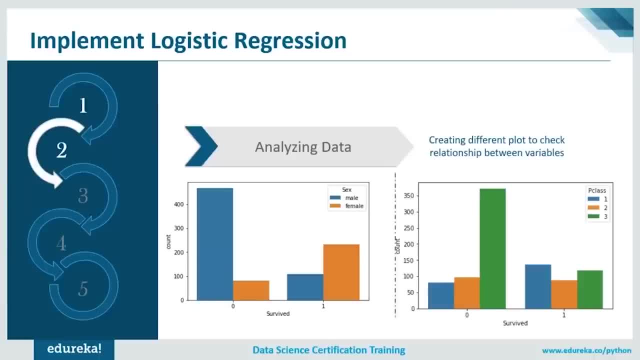 relationship between variables, as in how one variable is affecting the other. so you can simply explore your data set by making use of various columns and then you can plot a graph between them. So you can either plot a correlation graph, you can plot a distribution graph. 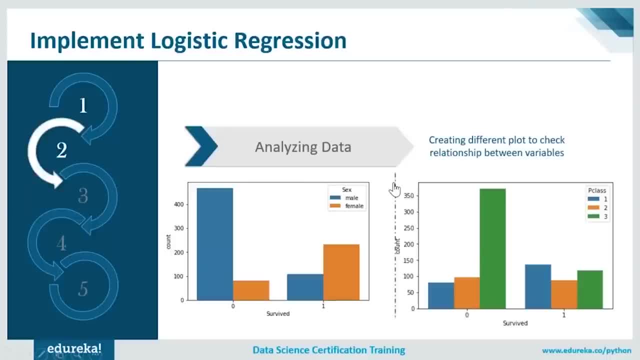 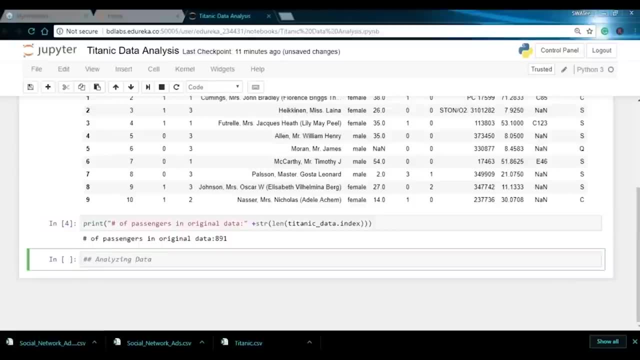 It's up to you guys. So let me just go back to my Jupyter Notebook and let me analyze some of the data over here. My second part is to analyze data. So I just put this in header to now. to put this in here to, I just 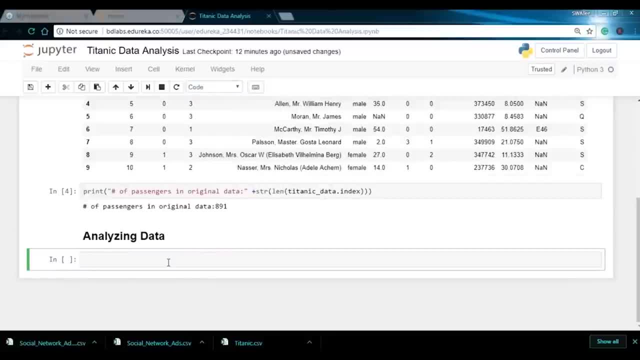 have to go on code, click on markdown and I just run this. suppose let us plot a count plot where you compare between the passengers who survived and who did not survive. So for that I'll be using the seaborn library. So over here I have imported seaborn as SNS. 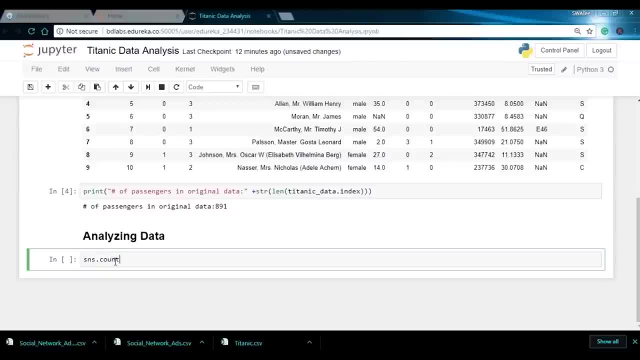 So I don't have to write the whole name and simply say SNS dot count plot. I'll say X is good to survive and the data that I'll be using is the Titanic data, or you can say the name of variable in which you have stored your data set. 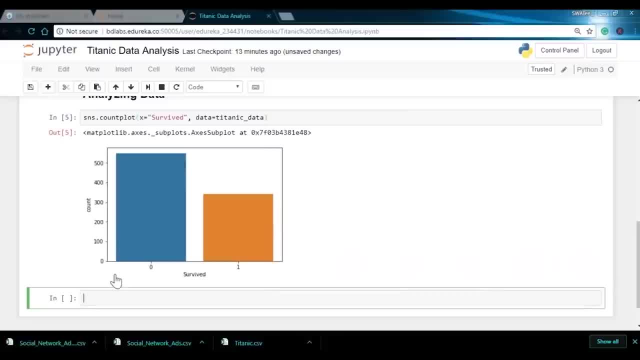 So now let me just run this. so over here, as you can see, I have survived column on my x-axis and on the y-axis I have the count. so zero basically stands for did not survive and one stands for the passengers who did survive over here. 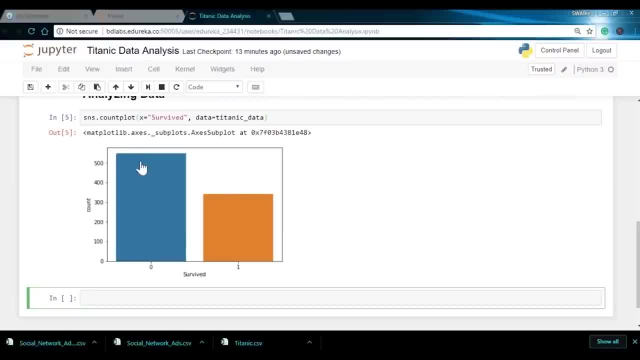 You can see that around 550 of the passengers who did not survive, and they were around 350 passengers Who only survive. So here you can basically conclude that there are very less survivors than non-survivors. So this was the very first plot. 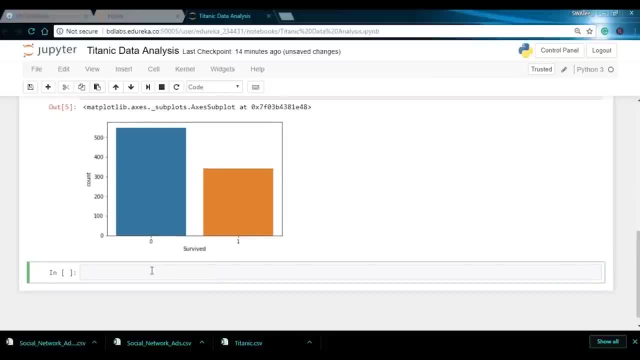 Now there is not another plot to compare the sex as to whether, out of all the passengers who survived and who did not survive, how many were men and how many were female. so to do that, I'll simply say: SNS dot count plot. I add the hue as sex. 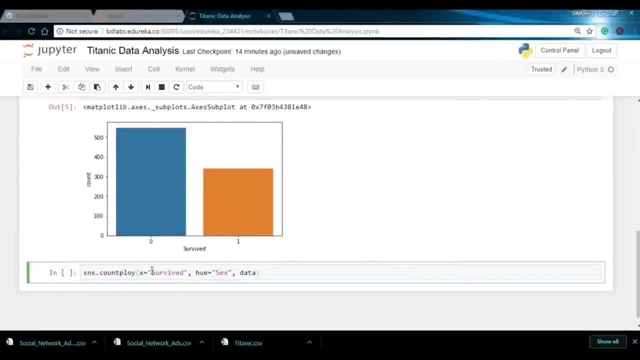 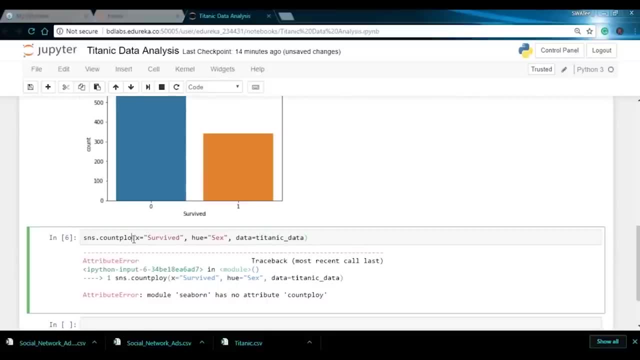 So I want to know how many females and how many males survive. then I'll be specifying the data. So I'm using Titanic data set and let me just run this. get done a mistake over here. over here You can see I have survived column on the x-axis and I have the 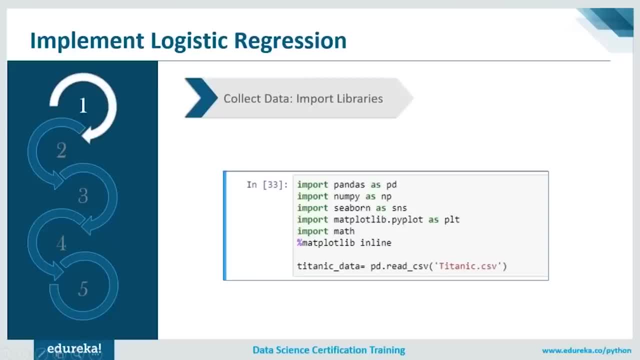 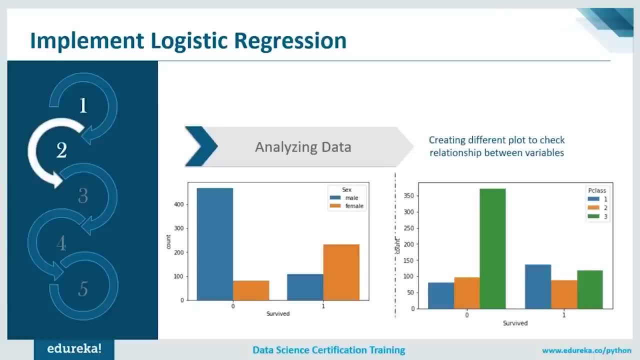 What is my next step? So we're done with the collecting data. next step is to analyze your data. So over here we'll be creating different plots to check the relationship between variables, as in variable is affecting the other. so you can simply explore your data. 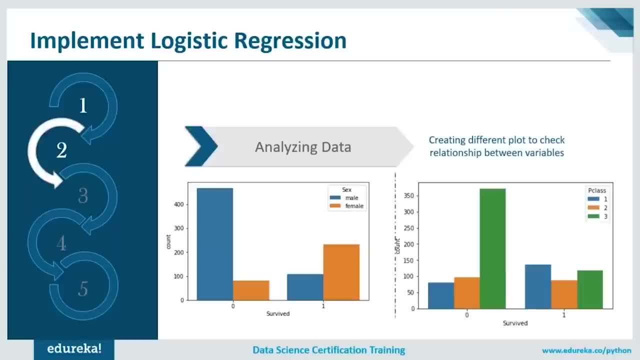 set by making use of various columns, and then you can plot a graph between them. So you can either plot a correlation graph, You can plot a distribution graph, It's up to you guys. So let me just go back to my Jupyter notebook and let me analyze. 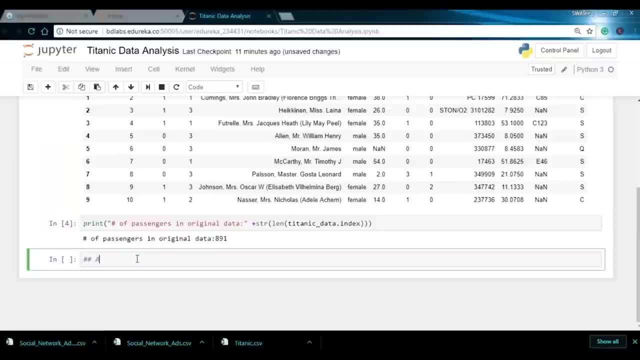 some of the data over here. My second part is to analyze data. So I just put this in header 2.. Now, to put this in header 2, I just have to go on code, click on markdown and I just run this. So first let us plot a count plot where you compare between the 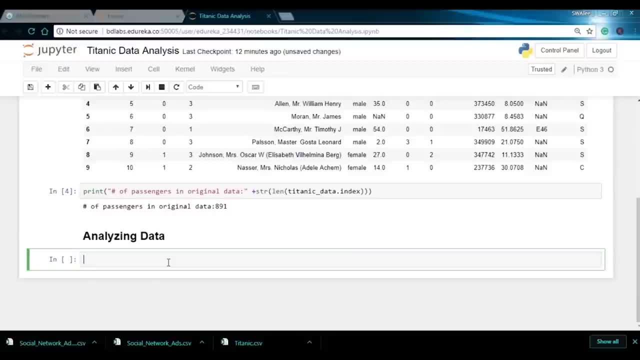 passengers who survive And who did not survive. So for that I'll be using the seabourn library. So over here I have imported seabourn as SNS, So I don't have to write the whole name. I'll simply say SNS dot count plot. 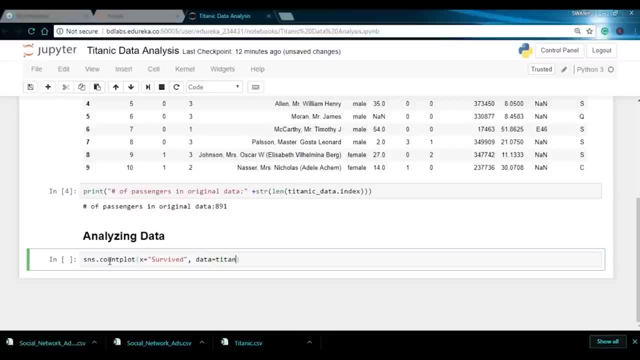 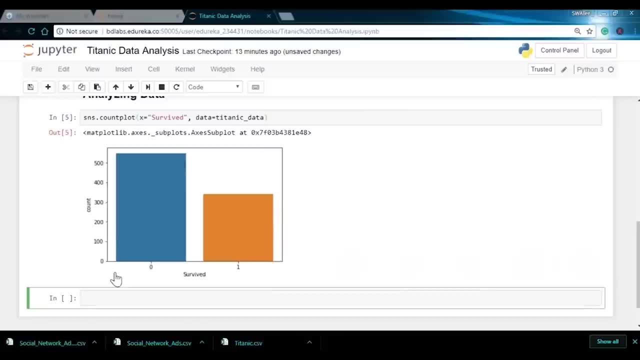 I'll say X is good to survive, and the data that I'll be using is the Titanic data, or you can say the name of variable in which you have stored your data set. So now let me just run this So over here. as you can see, I have survived column on my x-axis and 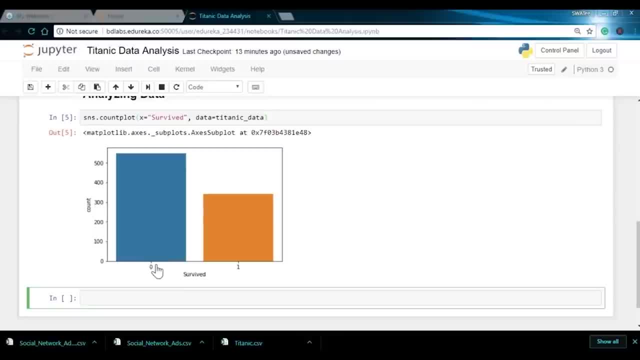 on the y-axis. I have the count. so zero basically stands for did not survive And one stands for the passengers who did survive. So over here you can see that around 550 of the passengers who did not survive and they were around 350 passengers who only survive. 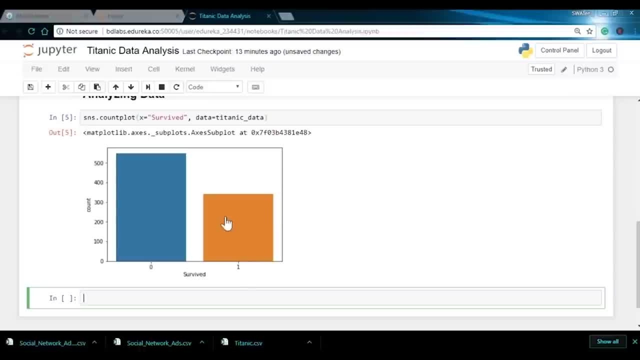 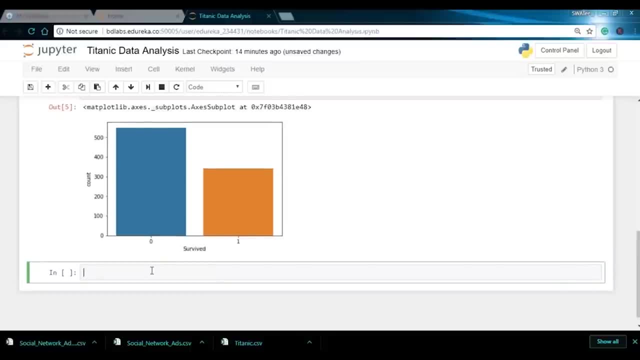 So here you can basically conclude that there are very less survivors than non-survivors. So this was the very first plot. Now let us plot another plot to compare the sex as to whether, out of all the passengers who survived and who did not survive, how many? 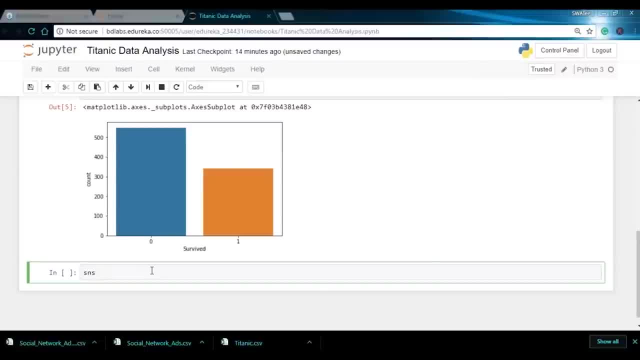 were men and how many were female. So to do that, I'll simply say SNS dot count plot. I add the hue as sex. So I want to know how many females and how many males survive. then I'll be specifying the data. 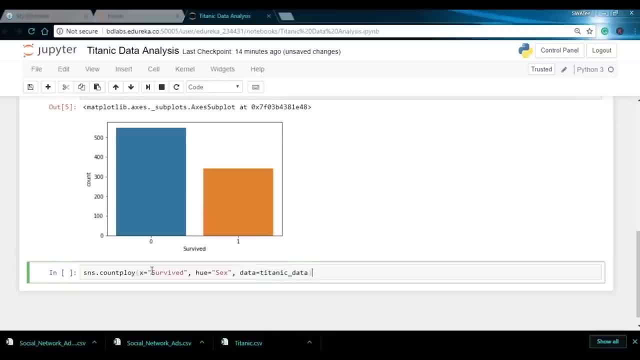 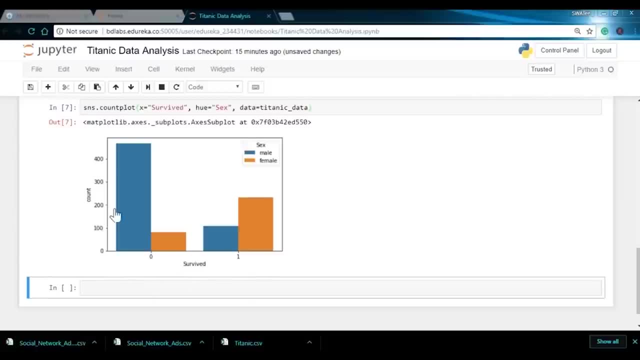 So I'm using Titanic data set and let me just run this. Okay, I've done a mistake over here, So over here you can see I have survived column on the x-axis and I have the count on the y now. So here your blue color stands for your male passengers, and orange. 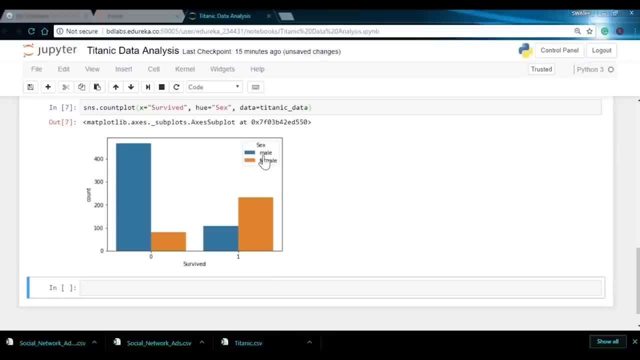 count on the wire now. So here your blue color stands for your male passengers and orange stands for your female. So, as you can see here, the passengers who did not survive, that has a value 0, so we can see that majority of males did not survive and 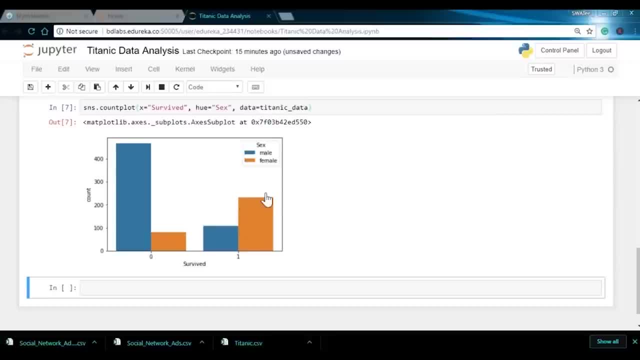 if we see the people who survived here, we can see the majority of female survive. So this basically concludes the gender of the survival rate. So it appears, on average women were more than three times more likely to survive than men. next Let us plot another plot where we have the hue as the passenger. 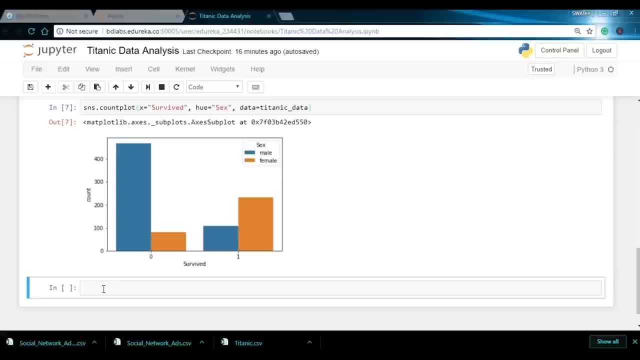 class. So over here we can see which class at the passenger was traveling in, whether it was traveling in class 1, 2 or 3.. So for that I just write the same command. I'll say SNS dot count plot. I'll keep my x-axis as something, only I'll change my hue to passenger. 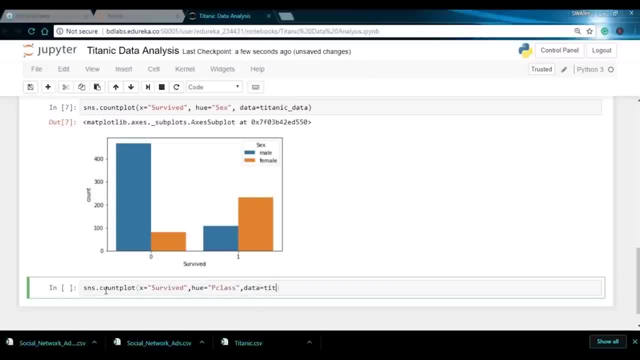 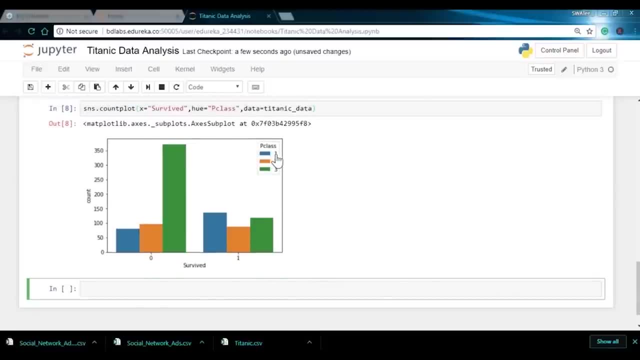 class. So my variable is named as P class And the data say that I'll be using this Titanic data. So this is my result. So over here you can see I have blue for first class, orange for second class and green for the third class. 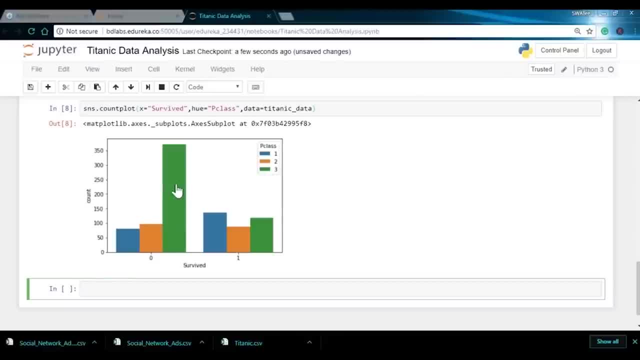 So here the passengers who did not survive were majorly of the third class, or you can say the lowest class or the cheapest class to get into the Titanic, and the people who did survive majorly belong to the higher classes. So here one and two has more rise than the passenger who were. 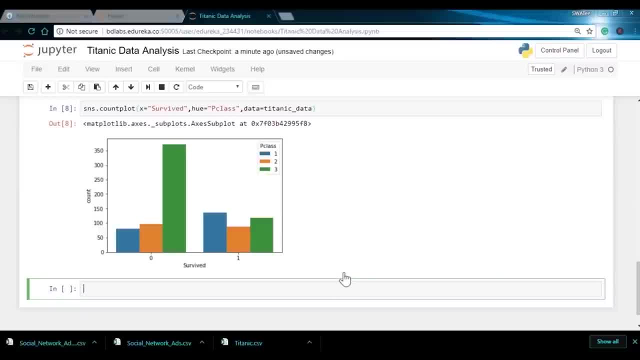 traveling in the third class. So here we have concluded that the passengers who did not survive were majorly of third class, or you can say the lowest class, and the passengers who were traveling in first and second class would tend to survive more. next, Let us plot a graph for the age distribution over here. 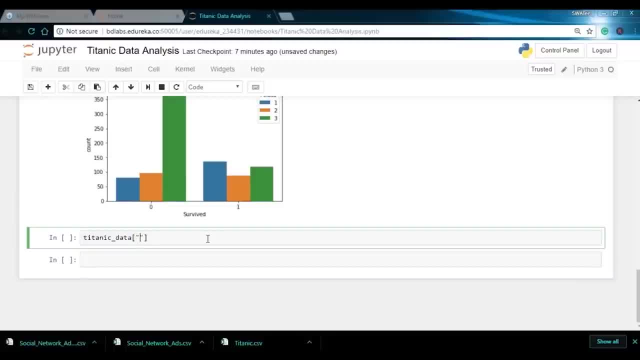 I can simply use my data. So we'll be using Pandas library for this. I'll declare an array and I'll pass in the column that is age. So I plot and I want a histogram, So I'll say: plot dot hist. 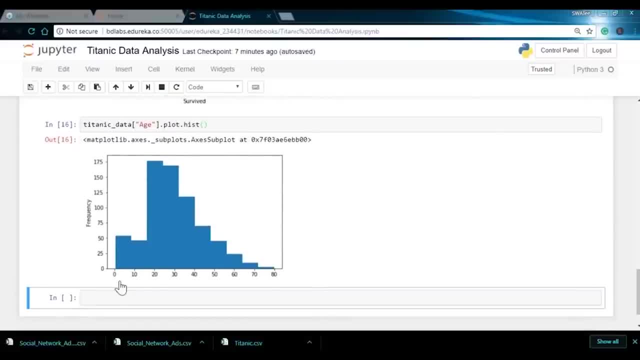 So you can notice over here that we have more of young passengers, or you can see the children between the ages 0 to 10, and then we have the average age people and if you go ahead, lesser would be the population. So this is the analysis on the age column. 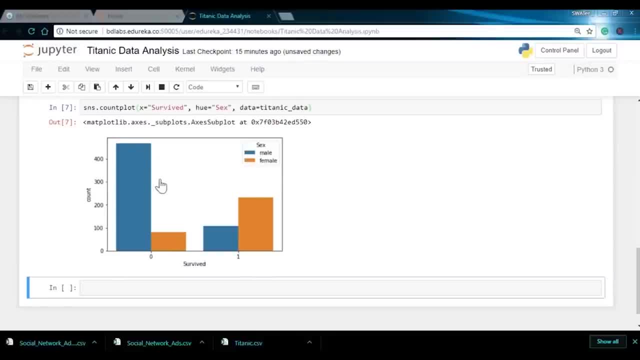 stands for your female. So, as you can see here the passengers who did not survive, that has a value Zero. So we can see that majority of males did not survive and if we see the people who survived here, we can see the majority of females. 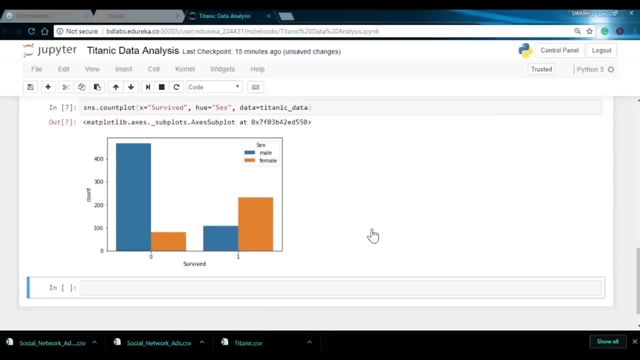 survive. So this basically concludes the gender of the survival rate. So it appears, on average, women were more than three times more likely to survive than men. Next, Let us plot another plot where we have the hue as the passenger class. So over here we can see which class that the passenger was traveling. 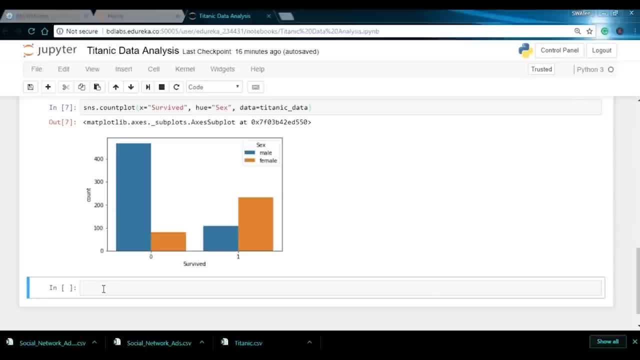 in whether it was traveling in class one, two or three. So for that I just write the same command. I'll say snscom- plot. I'll keep my x-axis as sub, only I'll change my hue to passenger class. So my variable is named as P class. 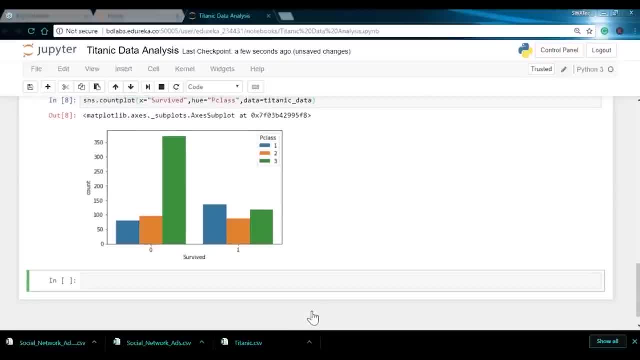 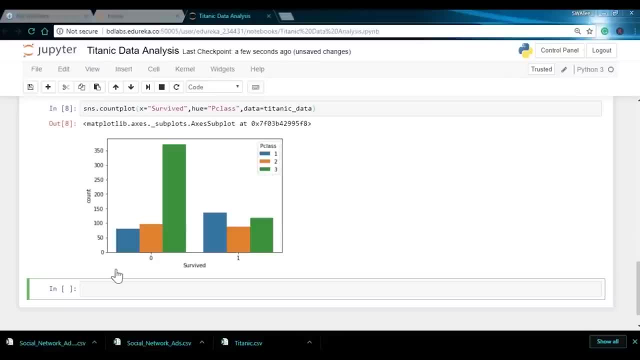 And the data say that I'll be using this Titanic data, So this is my result. So over here you can see I have blue for first class, orange for second class and green for the third class. So here the passengers who did not survive were majorly of the. 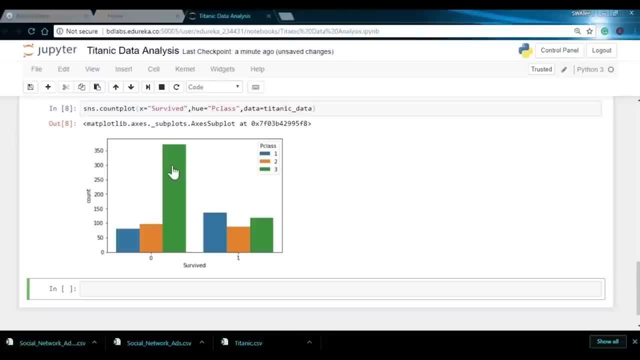 third class, or you can say the lowest class or the cheapest class to get into the Titanic, And the people who did survive majorly belong to the higher classes. So here one and two has more rise than the passenger who were traveling in the third class. 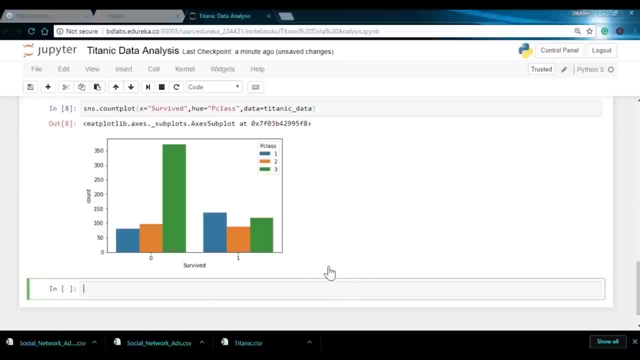 So here we have computed that the passengers who did not survive a majorly of third class, or you can say the lowest class, and the passengers who were traveling in first and second class would tend to survive more. Next, let us plot a graph for the age distribution over here. 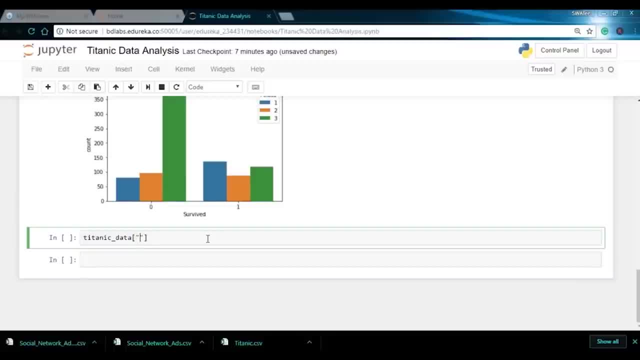 I can simply use my data. So we'll be using Pandas library for this. I'll declare an array and I'll pass in the column that is age. So I plot and I want a histogram, So I'll say: plot dot hist. 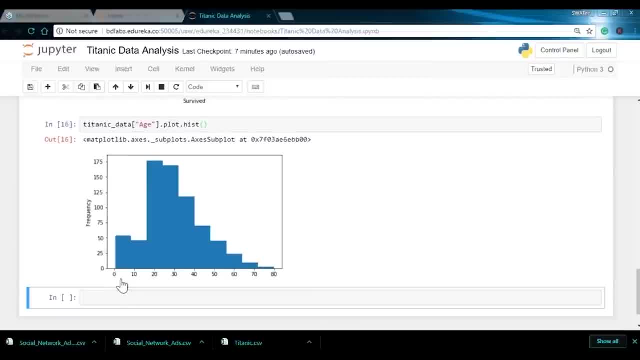 So you can notice over here that we have more of young passengers, or you can see the children between the ages 0 to 10, and then we have the average age people and if you go ahead, lesser would be the population. So this is the analysis on the age column. 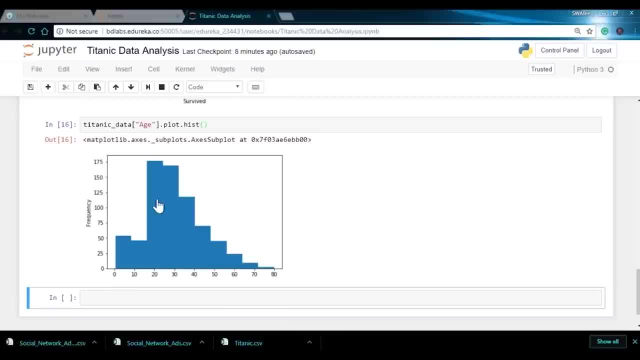 So we saw that we have more young passengers and more mediocre age passengers which are traveling in the Titanic. So next, let me plot a graph of air as well. So I'll say Titanic data, I'll say fair and again I'll plot a histogram. 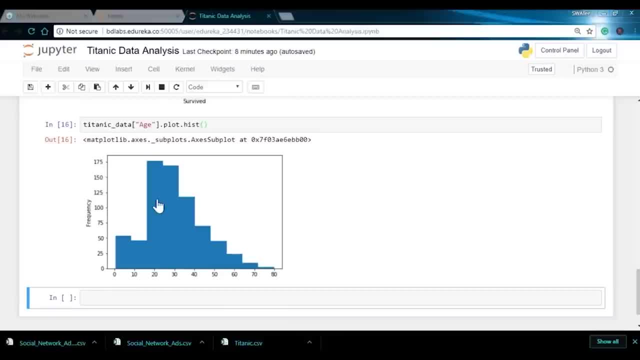 So we saw that we have more young passengers and more mediocre age passengers which are traveling in the Titanic. So next, let me plot a graph of air as well. So I'll say Titanic data, I'll say fair And again I'll plot a histogram. 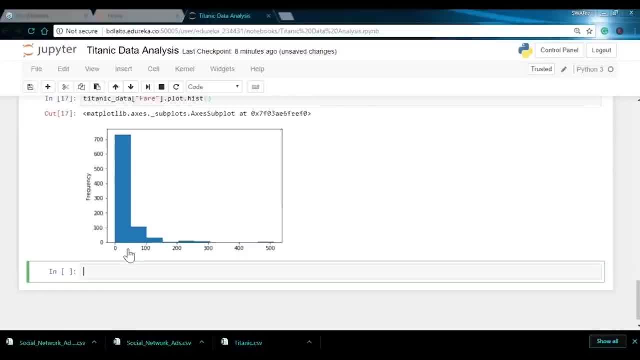 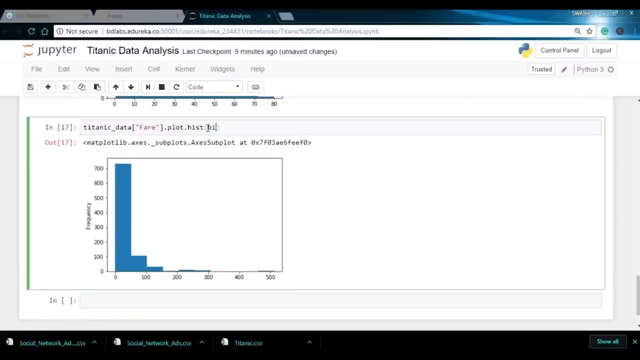 So I'll say hist. So here you can see. the fair size is between 0 to 100.. Now let me add the bin size, so as to make it more clear over here. I'll say: bin is equals to, let's say, 20, and I'll increase the figure. 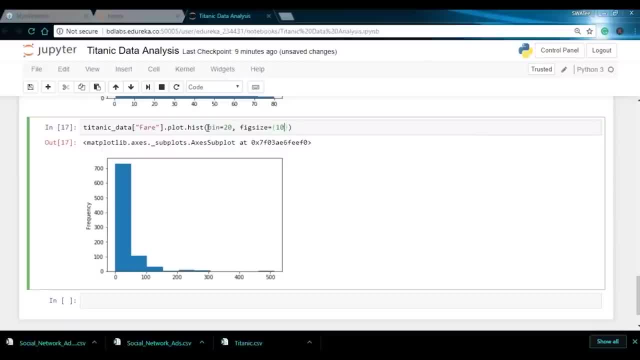 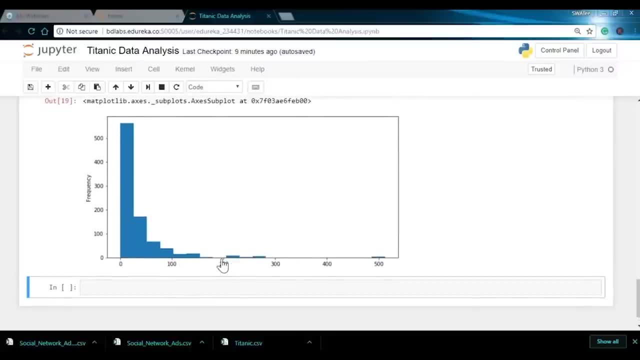 size as well. So I'll say fixed size. Let's say I give the dimensions as 10 by 5. So it is bins. So this is more clear now. Next, Let us analyze the other columns as well. So I'll just type in Titanic data. 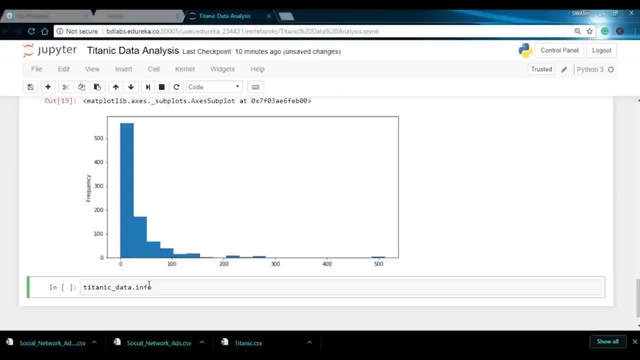 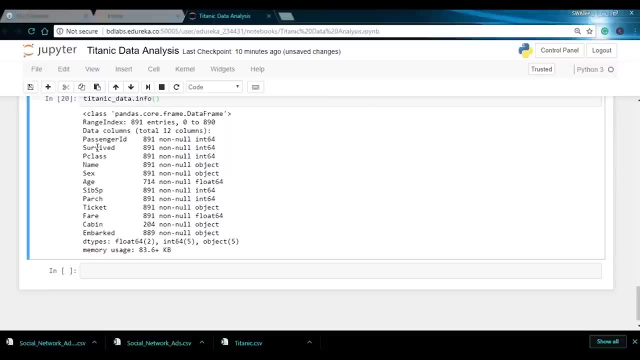 And I want the information as to what all columns are left. So here we have passenger ID, which I guess it's of no use. Then we have see how many passengers survive and how many did not. We also see the analysis on the gender basis. 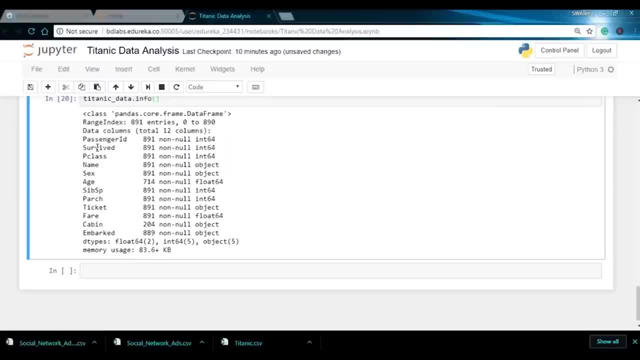 We saw when the female tend to survive more or the men tend to survive more. Then we saw the passenger class, where the passenger is traveling in the first class, second class or third class. Then we have the name. So in name we cannot do any analysis. 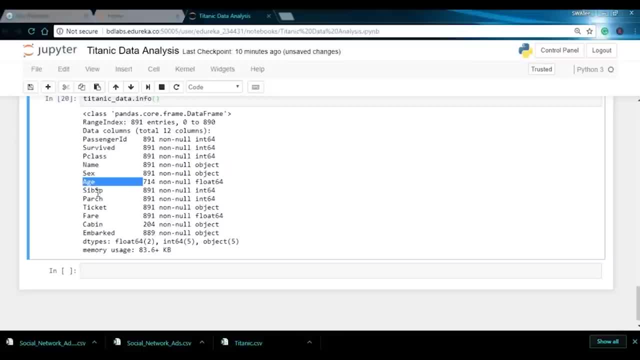 We saw the sex, we saw the age as well. Then we have Sib, SP. So this stands for the number of siblings, or the spouses, which are aboard the Titanic. So let us do this as well. So I'll say snscom plot. 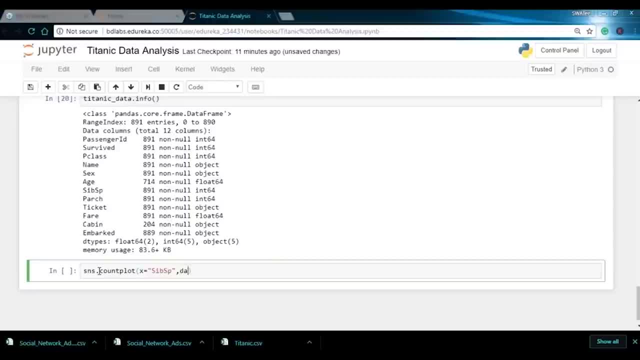 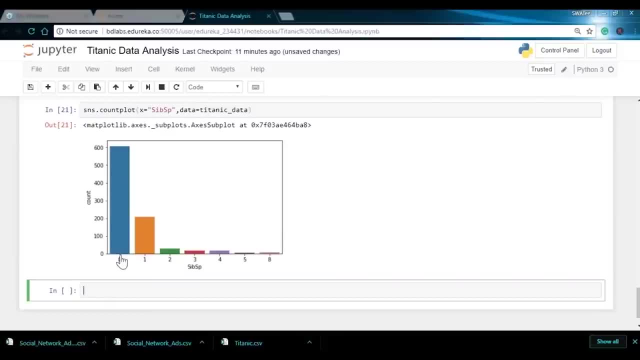 I'll mention X as Sib SP And I'll be using the Titanic data So you can see the plot over here. So over here you can conclude that it has the maximum value on zero. So you can conclude that neither a children nor a spouse was. 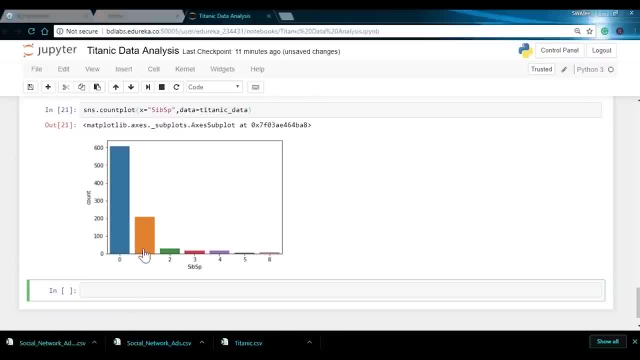 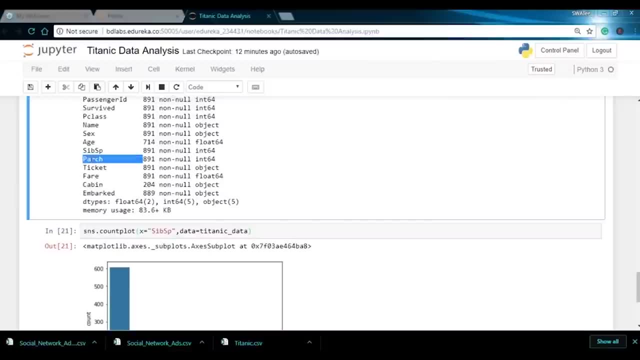 on board the Titanic. Now, second most highest value is one, And then we have very less values for two, three, four and so on. Next, if I go above- we saw this column as well- similarly can do for part, So next we have part, or you can say the number of parents or 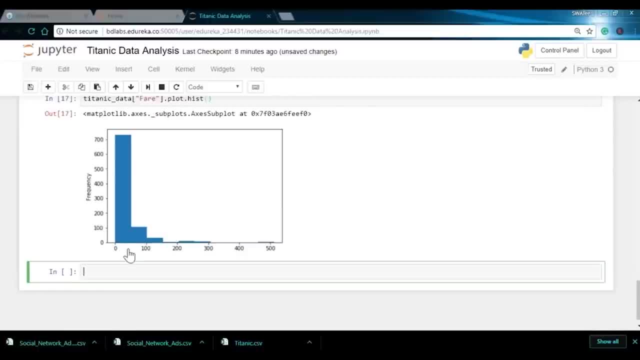 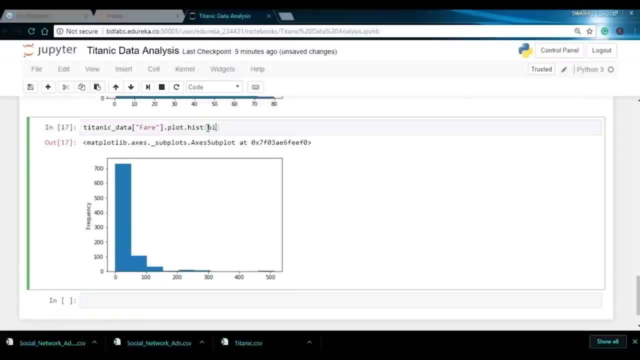 So I'll say hist. So here you can see. the fair size is between 0 to 100.. Now let me add the bin size, so as to make it more clear over here. I'll say: bin is equals to, let's say, 20, and I'll increase the figure. 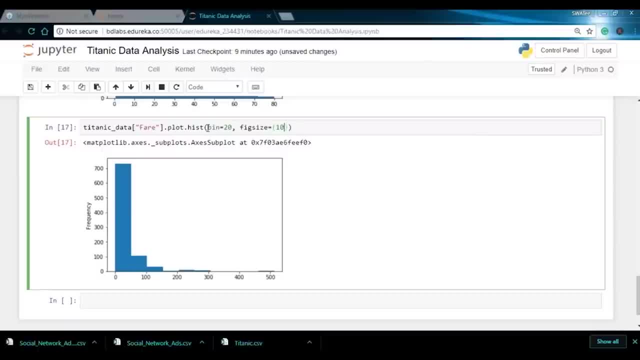 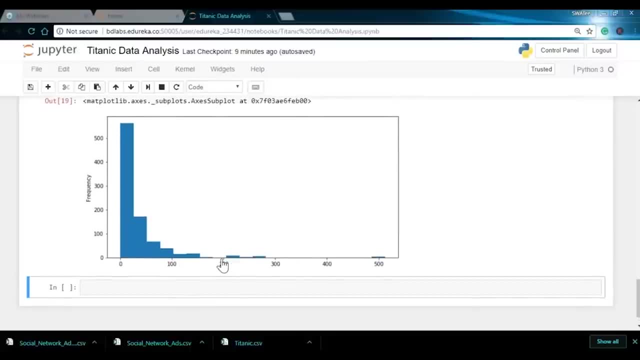 size as well. So I'll say fixed size. Let's say I give the dimensions as 10 by 5. So it is bins. So this is more clear now. Next, let us analyze the other columns as well. So I'll just type in Titanic data, and I want the information as 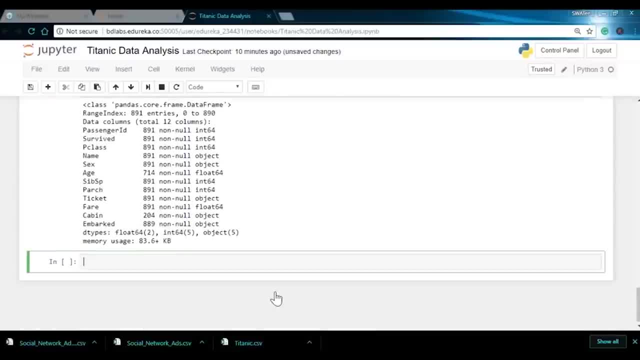 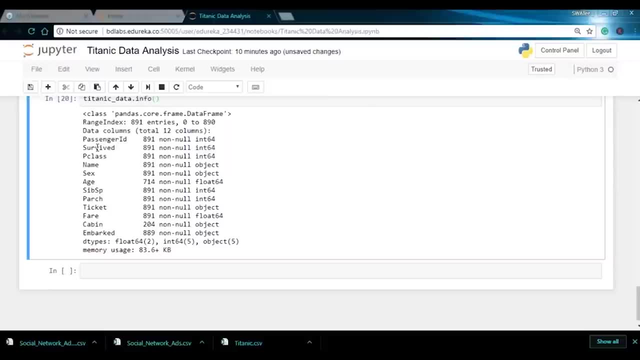 to what all columns are left. So here we have passenger ID, which I guess it's of no use. then we have see how many passengers survived and how many did not. we also see the analysis on the gender basis. We saw when the female tend to survive more or the men tend to. 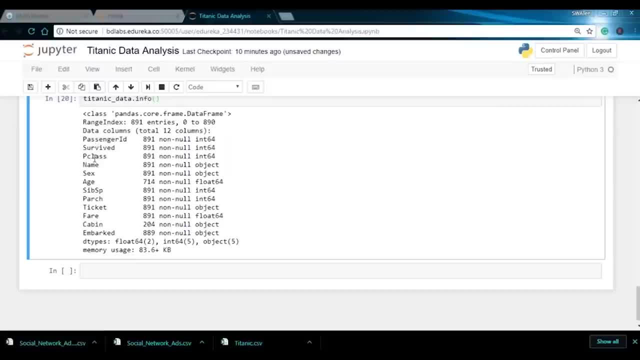 survive more. then we saw the passenger class, where the passenger is traveling in the first class, second class or third class. then we have the name. So in name We cannot do any analysis. We saw the sex. We saw the age as well. Then we have Sib SP. 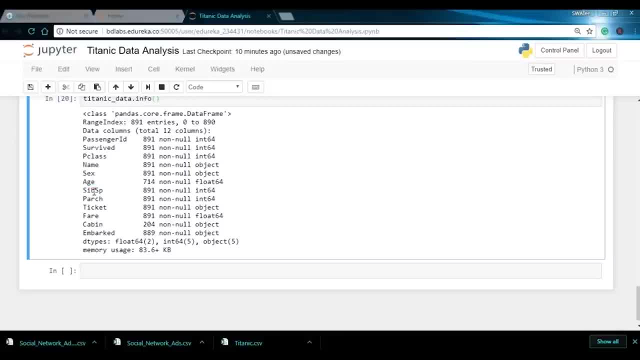 So this stands for the number of siblings, or the spouses, which are aboard the Titanic. So let us do this as well. So I'll say snscom plot, I'll mention X as Sib, SP And I'll be using the Titanic data. 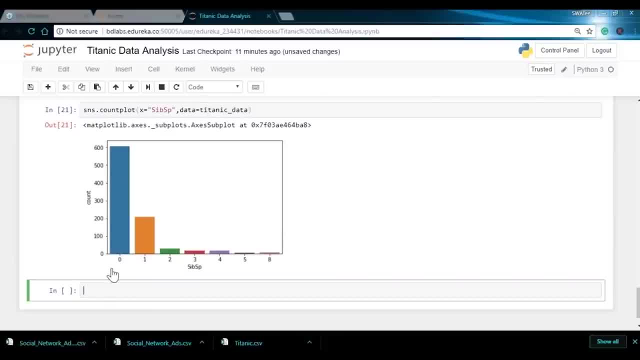 So you can see the plot over here. So over here you can conclude that it has the maximum value on 0. so you can conclude that neither Nor a spouse was on board the Titanic. Now, second most highest value is 1, and then we have very less values. 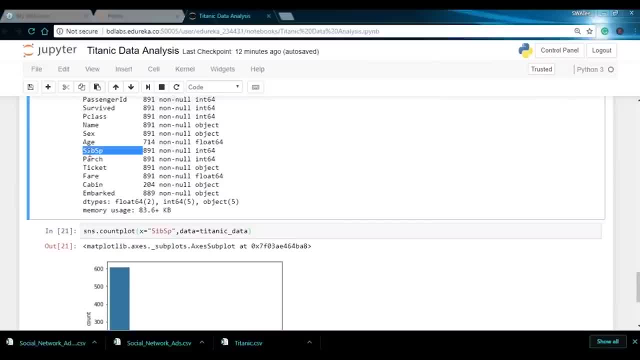 for 2, 3, 4 and so on. next, if I go above, we saw this column as well. Similarly, you can do for parts, So next we have parts. or you can say the number of parents or children which were aboard the Titanic. So you, similarly, can do this as well. 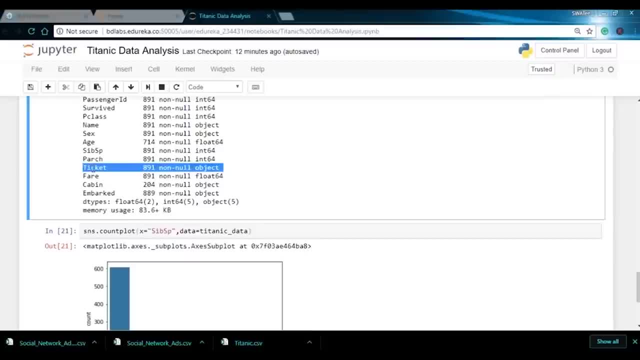 Then we have the ticket number. So I don't think so any analysis is required for ticket. Then we have fair, so fair. We have already discussed as in the people who tend to travel in the first class, You will pay the highest fair. then we have the cabin number and we 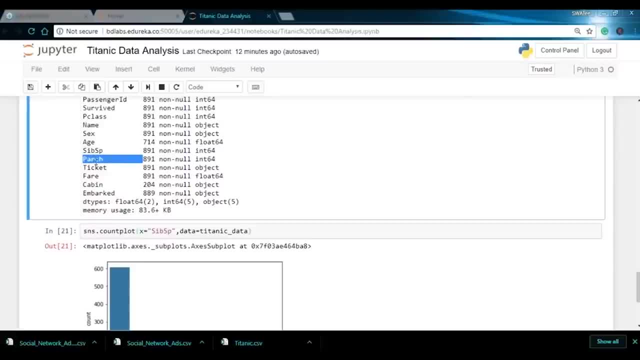 children which were aboard the Titanic, So you, similarly, can do this as well. Then we have the ticket number. So I don't think so Any analysis is required for ticket. Then we have fair, so fair. We have already discussed, as in the people who tend to travel, 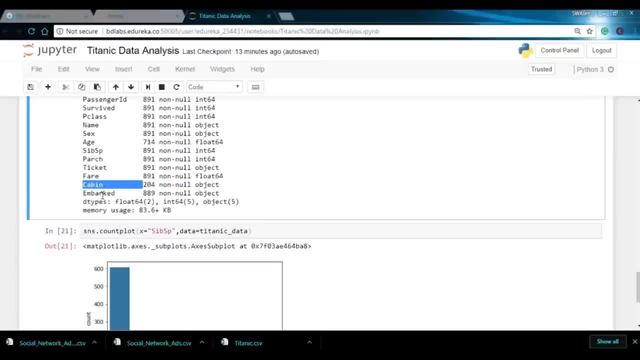 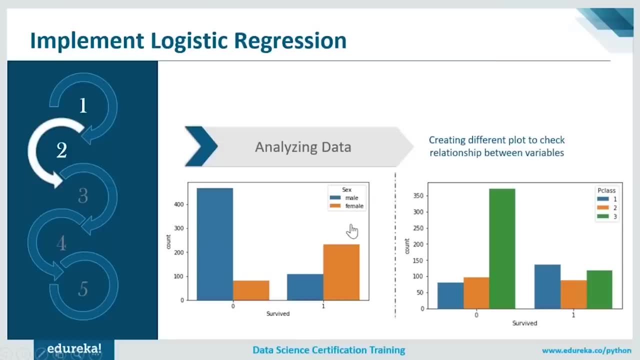 in the first class usually pay the highest fare. Then we have the cabin number and we have embarked. So these are the columns That will be doing data wrangling on. so we have analyzed the data and we have seen quite a few graphs in which we can. 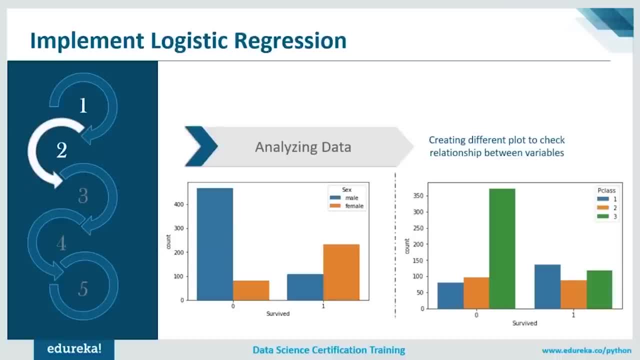 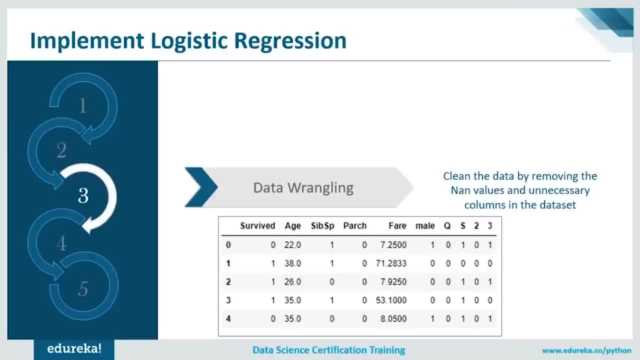 conclude which variable is better than the another or what is the relationship they hold. So third step is my data wrangling. So data wrangling basically means cleaning your data. So if you have a large data set, you might be having some null values or you can say any and values. 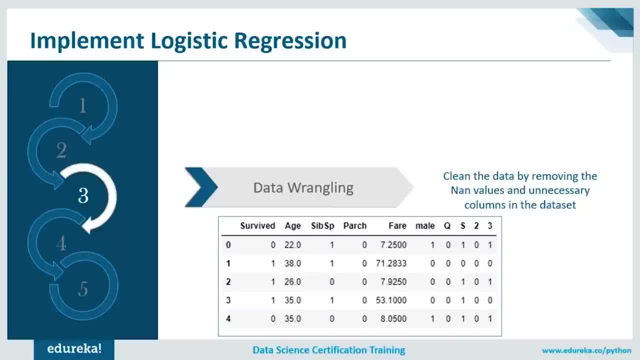 So it's very important that you remove all the unnecessary items that are present in your data set. So removing this directly affects your accuracy. So I'll just go ahead and clean my data. We're removing all the nan values and unnecessary columns, which has a null value in the data set. 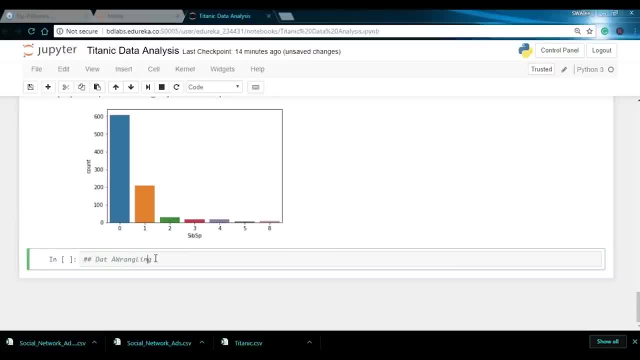 So next I'll be performing data wrangling. So first of all I'll check whether my data set is null or not. So I'll say Titanic data, which is the name of my data set, and I'll say is null. So this will basically tell me what all values are null. 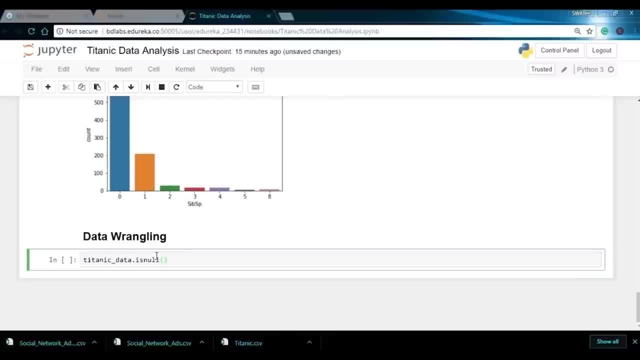 and it will return me a boolean result. So this basically checks the missing data and your result will be in boolean format. Then the result will be true or false. So false mean if it is not null and true means if it is null. So let me just run this. 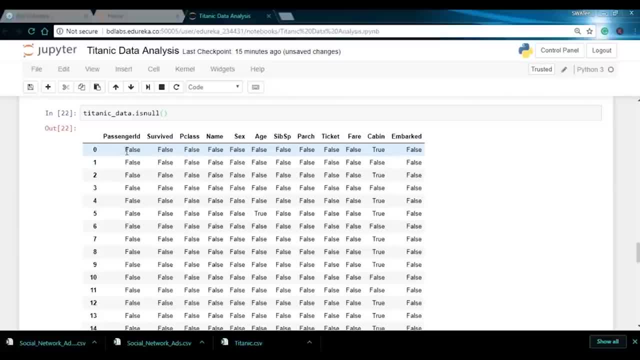 Over here you can see the values as false or true. So false is where the value is not null and true is where the value is null. So over here you can see, in the cabin column We have the very first value, which is null. 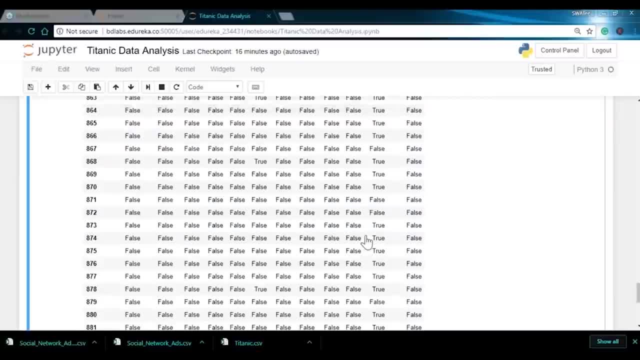 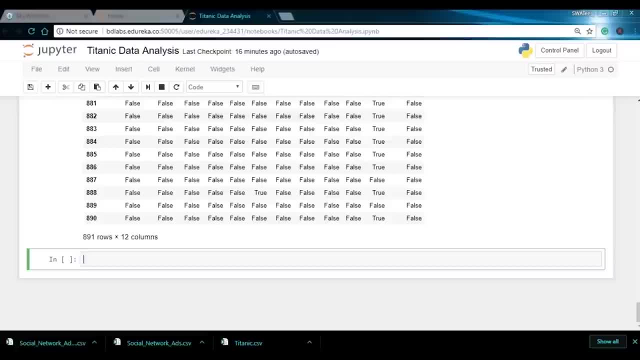 So we have to do something on this So you can see that we have a large data set, So the counting does not stop and we can actually see the sum of it. We can actually print the number of passengers who have the NAN value in each column. 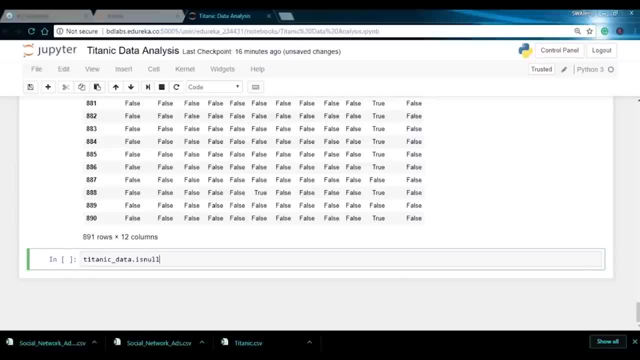 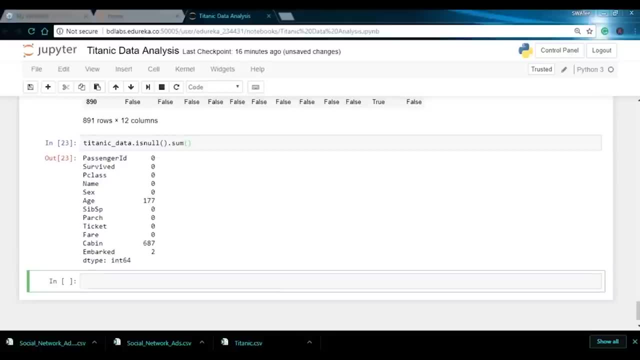 So I'll say Titanic underscore data is null and I want the sum of it, So I'll say dot sum. So this will basically print the number of passengers who have the NAN values in each column. So we can see that we have missing values in each column. 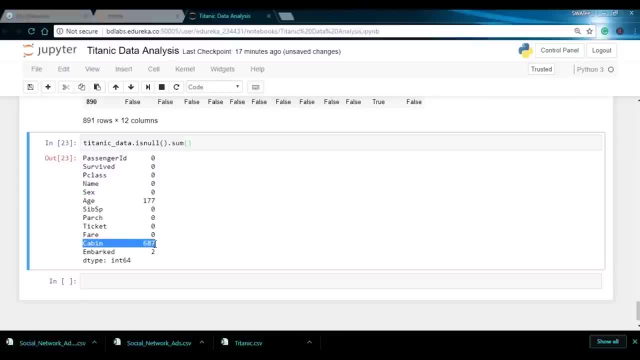 That is 177.. Then we have the maximum value in the cabin column and we have very less in the impact column, That is 2.. So here, if you don't want to see this numbers, you can also plot a heat map and then you can visually analyze. 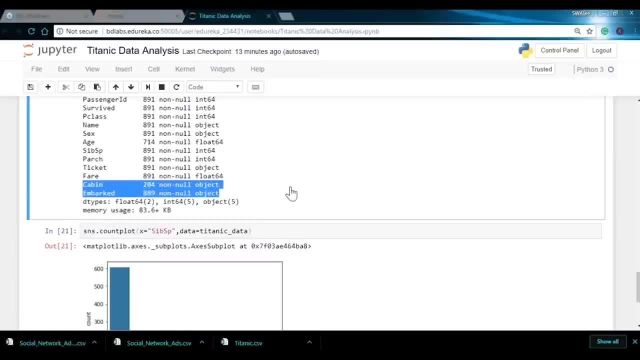 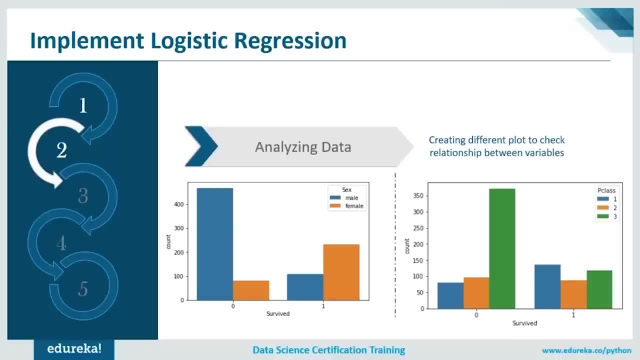 have embarked. So these are the columns that we'll be doing data wrangling on. So we have analyzed the data and we have seen quite a few graphs in which we can conclude which variable is better than the another or what is the relationship they hold. 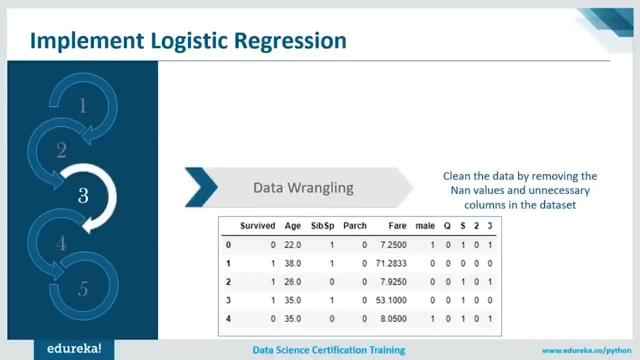 So third step is my data wrangling. So data wrangling basically means cleaning your data. So if you have a large data set, you might be having some null values or you can say any and values. So it's very important that you remove all the unnecessary items that 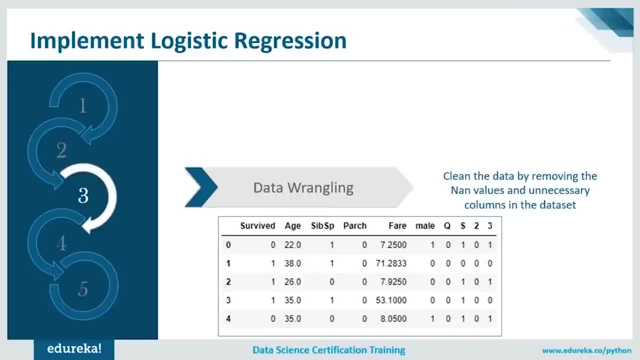 are present In your data set, So removing this directly affects your accuracy. So I'll just go ahead and clean my data by removing all the NN values and unnecessary columns, which has a null value in the data set. So next I'll be performing data wrangling. 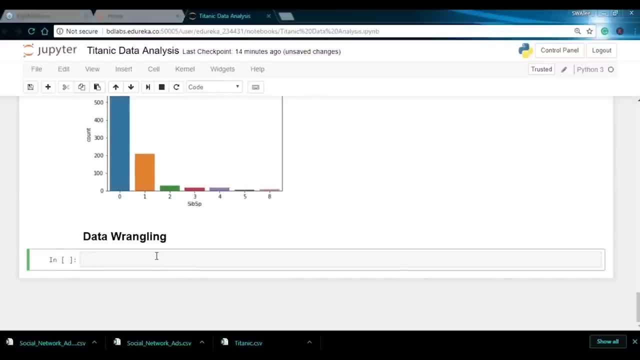 So first of all, I'll check whether my data set is null or not. So I'll say Titanic data, which is the name of my data set, and I'll say is null. So this will basically tell me what. all values are null and it will return. 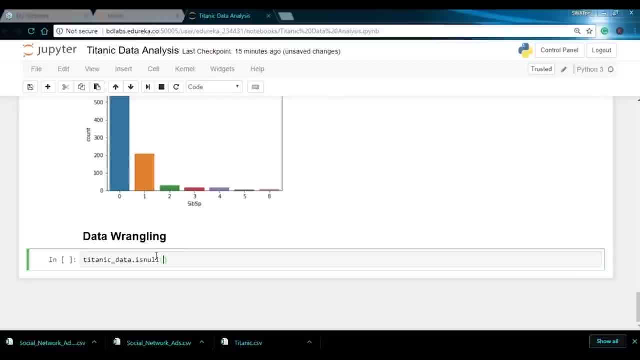 me a boolean result. So this basically checks the missing data and your result will be in boolean format as in. the result will be true or false. So false mean if it is not none and true means if it is null. So let me just run this. 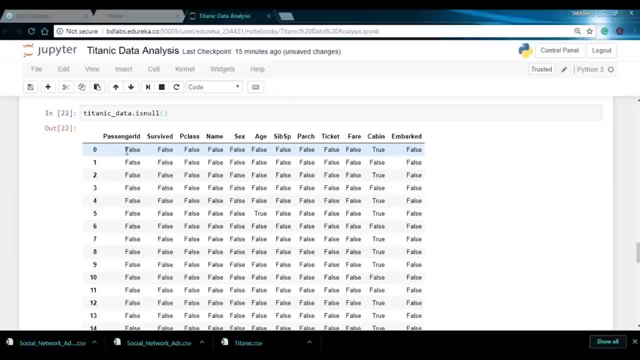 Over here you can see the values as false or true. So false is where the value is not null and true is where the value is none. So over here you can see, in the cabin column We have the very first value, which is null. 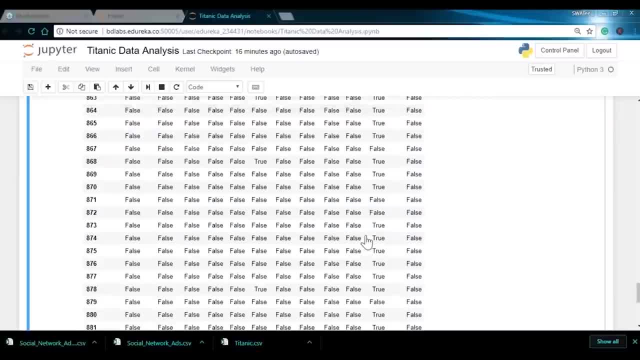 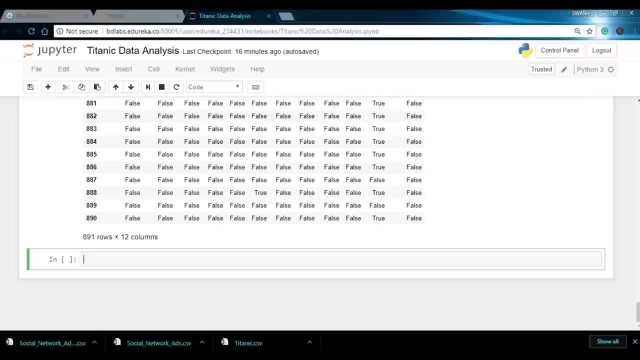 So we have to do something on this so you can see that we have a large data set, The counting does not stop and we can actually see the sum of it. We can actually print the number of passengers who have the NAN value in each column. 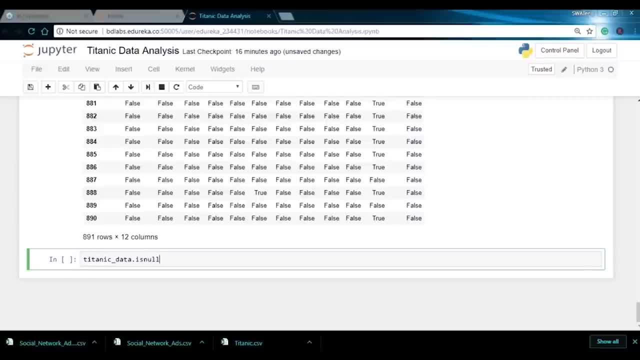 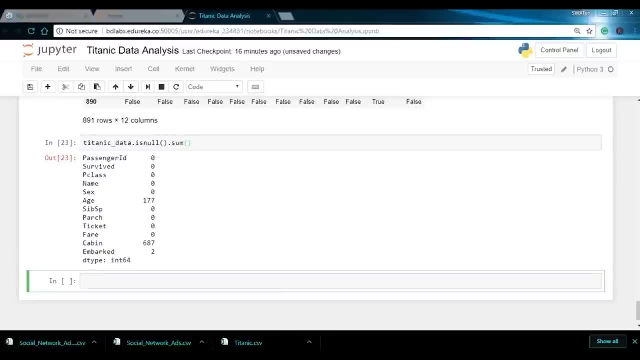 So I'll say Titanic underscore data is null and I want the sum of it. Well, say dot sum. So this will basically print the number of passengers who have the NAN values in each column. So we can see that we have missing values in each column. 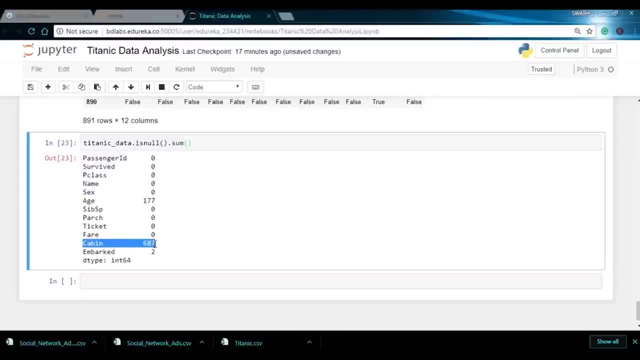 That is 177.. Then we have the maximum value in the cabin column and we have very less in the impact column, That is 2.. So here, if you don't want to see this numbers, you can also plot a heat map and then you can visually analyze it. 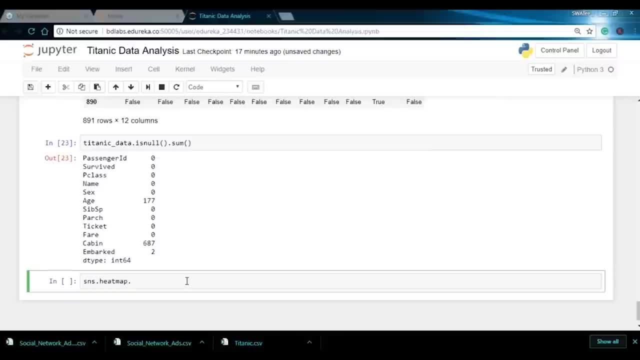 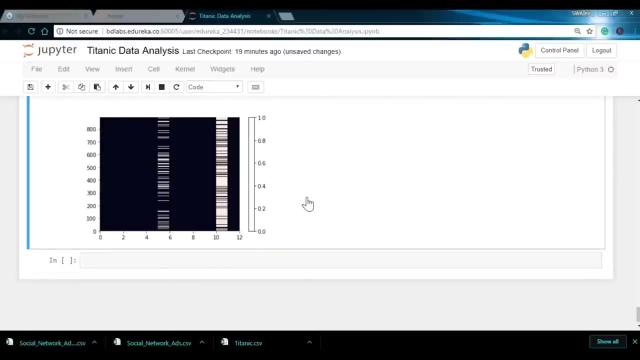 So let me just do that as well. So I'll say SNS dot heat map, I'll say why tick labels Falls. So I'll just run this so, as we have already seen that there were three columns in which missing data value was present, 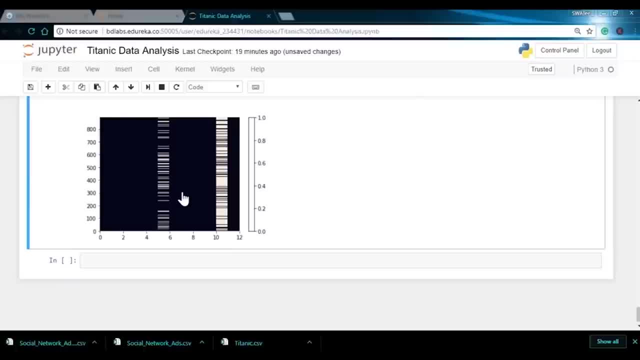 So this might be age. So over here almost 20% of age column has a missing value. Then we have the keeping columns, So this is quite a large value, and then we have two values for embark column as well. Add a C map for color coding. 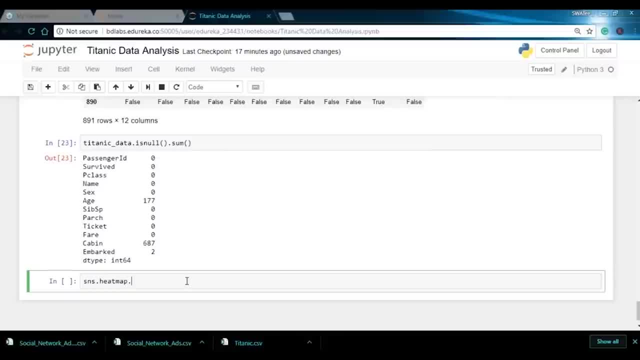 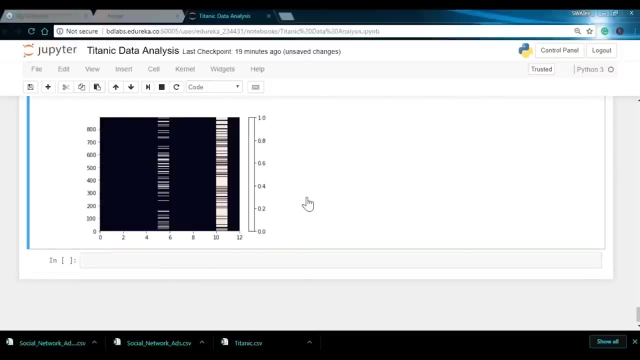 It. let me just do that as well. So I'll say SNS dot heat map. I'll say why tick labels falls. So I'll just run this. So, as we have already seen that there were three columns in which missing data value was present, 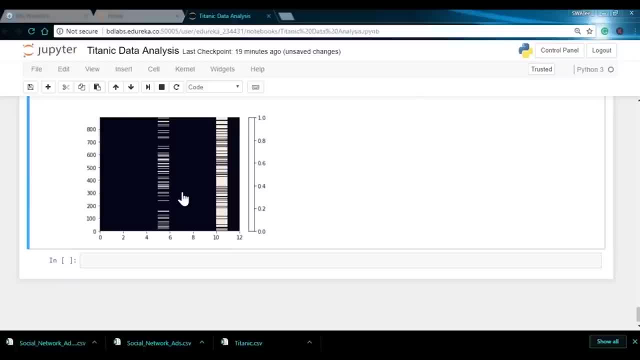 So this might be age. So over here, almost 20% of age column has a missing value. Then we have the caping columns. So this is quite a large value, and then we have two values for impact column as well. Add a C map for color coding. 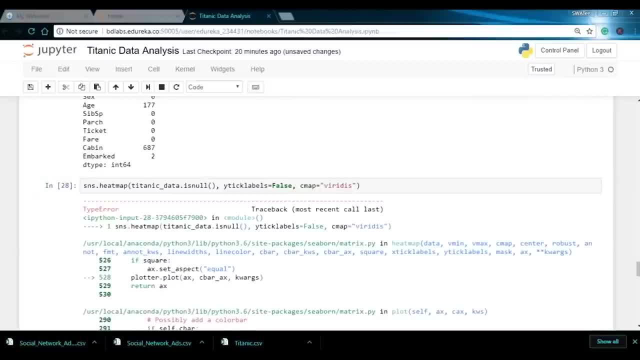 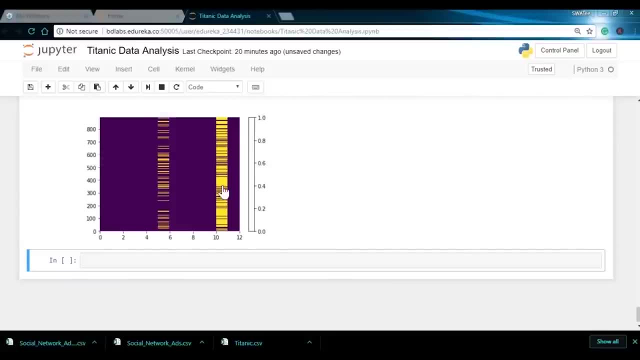 So I'll say C map. So if I do this, so the graph becomes more attractive. So over here your yellow stands for true, or you can say the values are null. So here we have concluded that we have the missing value of age. 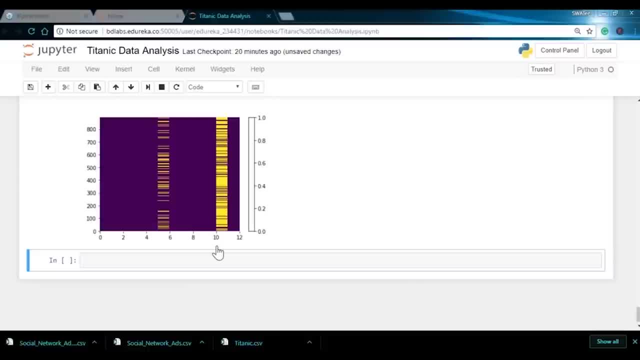 We have a lot of missing values in the cabin column and we have very less value which is not even visible in the embark column as well. So to remove these missing values, you can either replace the values and you can Send some dummy values to it, or you can simply drop the column. 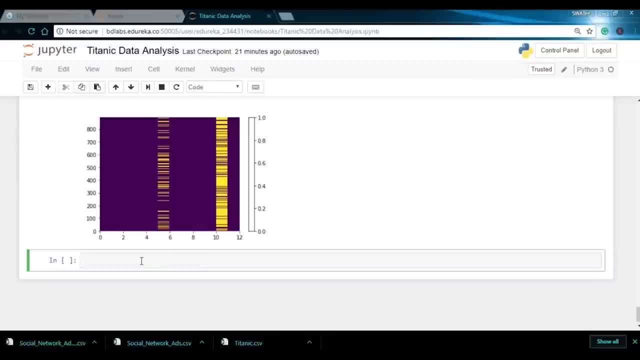 So here let us first pick the age column. So first let me just plot a box plot and they will analyze with having a column as age. So I'll say SNS dot box plot. I'll say X is equals to passenger class, So it's P class. 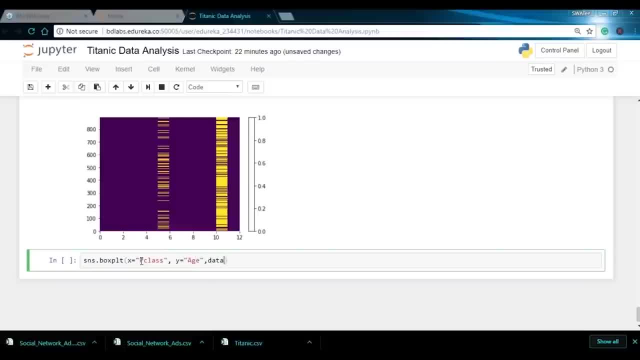 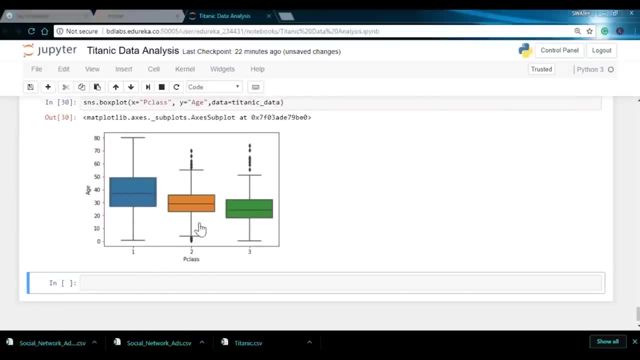 I'll say Y is equals to age and the data set that I'll be using is Titanic set. So I'll say data is equals to Titanic data. You can see the age in first class and second class tends to be more older, rather than we have it in the third class. 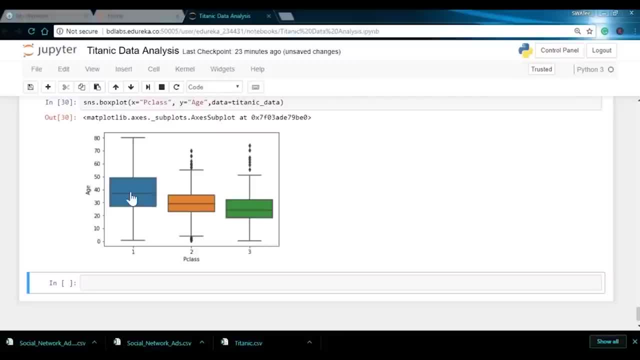 Well, that depends on the experience, how much you earn or might be. there n number of reasons. So here we concluded that passengers who were traveling in class 1 and class 2 attend to be older than what we have in the class 3.. So we have found that we have some missing values in M. 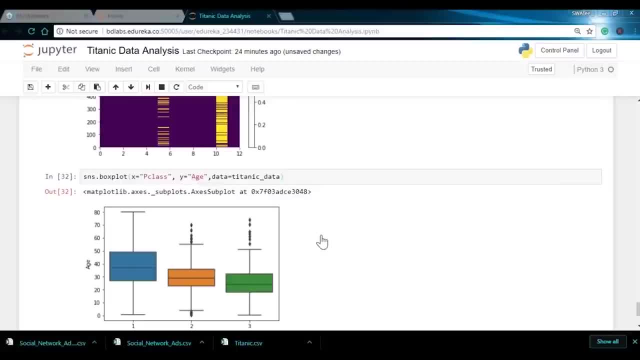 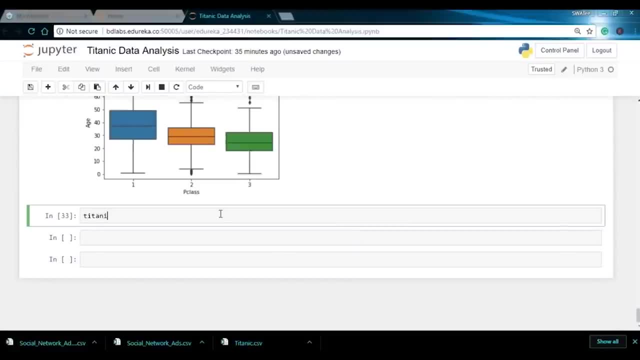 Now one way is to either just drop the column or you can just simply fill in some values to them. So this method is called as imputation. now to perform data wrangling or cleaning, Let us first print the head of the data set. So I'll say Titanic, not head. 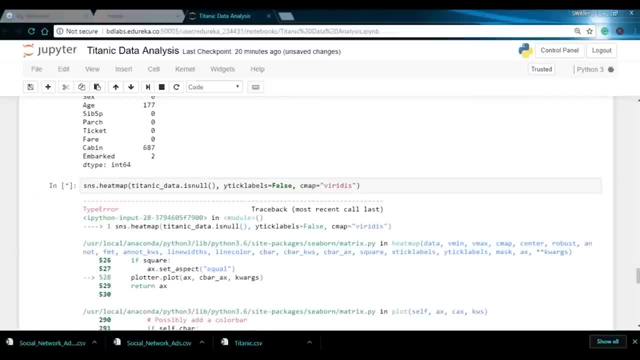 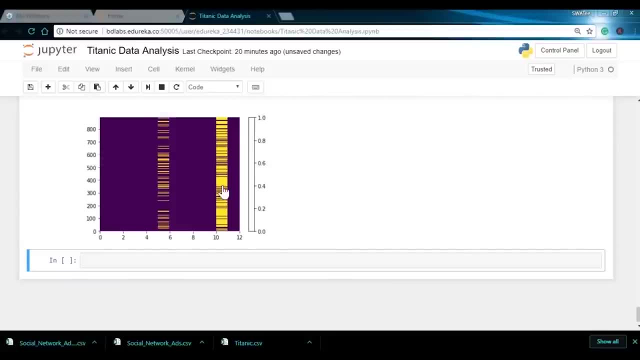 So I'll say C map. So if I do this, so the graph becomes more attractive. So over here your yellow stands for true, or you can say the values are null. So here we have concluded that we have the missing value of age. 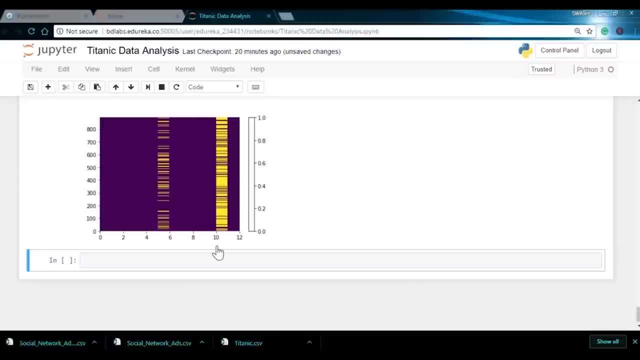 We have a lot of missing values in the cabin column and we have very less value which is not even visible In the embark column as well. So to remove these missing values, you can either replace the values and you can put in some dummy values to it, or you can simply drop the column. 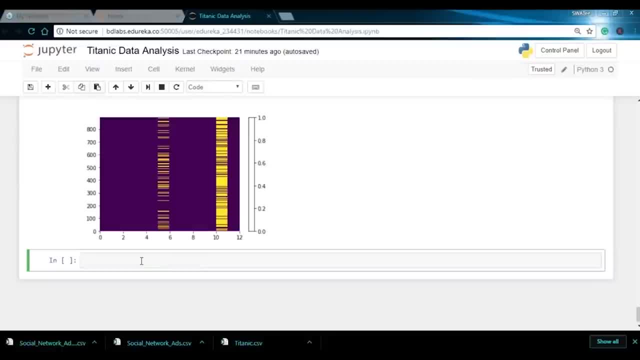 So here let us first pick the age column. So first let me just plot a box plot and they will analyze with having a column as age. So I'll say SNS dot box plot. I'll say X is equals to passenger class, So it's P class. 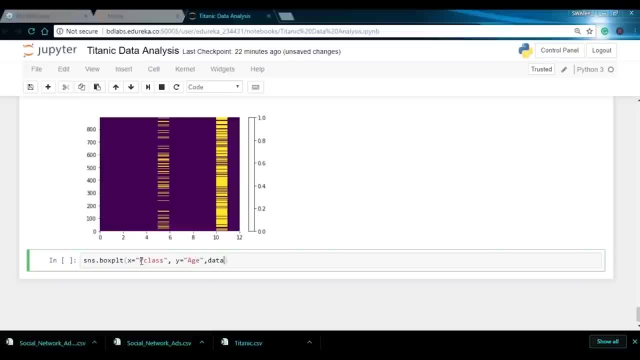 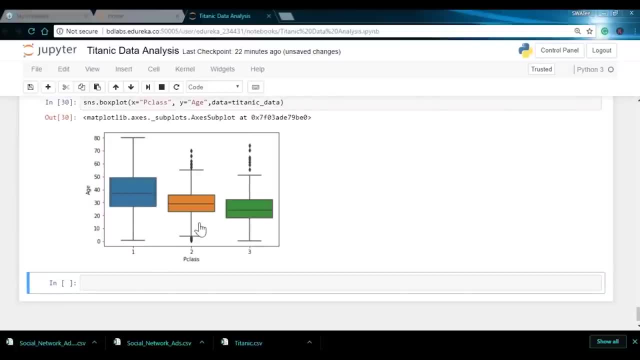 I'll say Y is equals to age and the data set that I'll be using is Titanic set. So I'll say data is equals to Titanic data. You can see the age in first class and second class tends to be more older, rather than we have it in the third class. 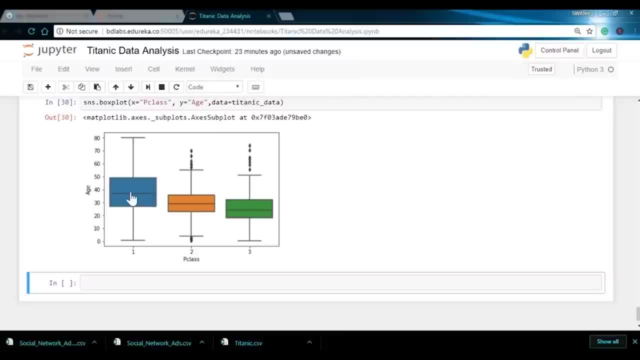 Well, that depends on the experience, how much you earn or might be. there n number of reasons. So here we concluded that passengers who were traveling in class 1 and class 2 are tend to be older than what we have in the class 3.. 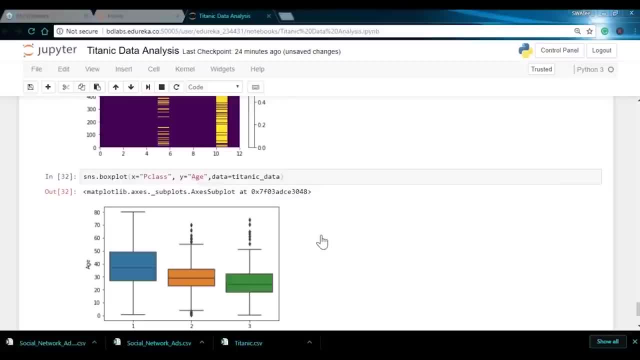 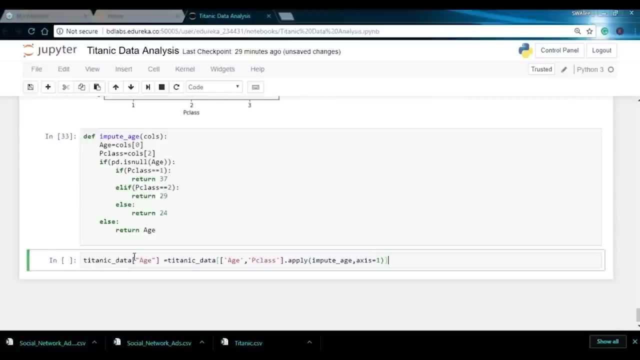 So we have found that we have some missing values in M. Now one way is to either just drop the column or you can just simply fill in some values to them. So this method is called as imputation. Now to perform data wrangling or cleaning: 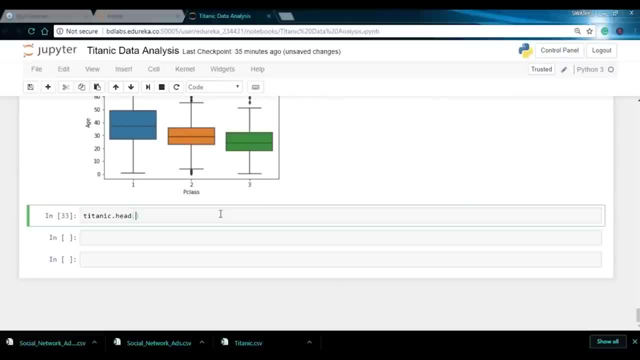 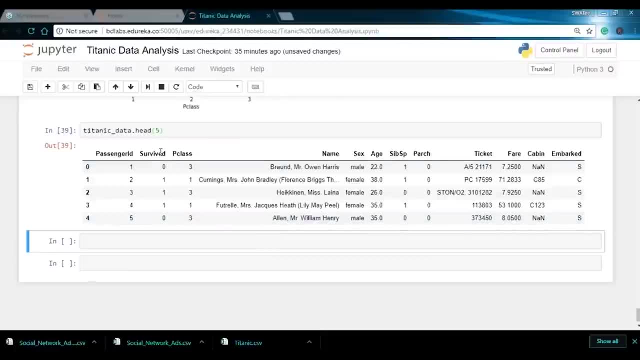 Let us first print the head of the data set. So I'll say Titanic, not head, So it's Titanic underscore data. Let's say: I just want the five rows. So here we have survived, which is again categorical. So in this particular column I can apply logistic regression. 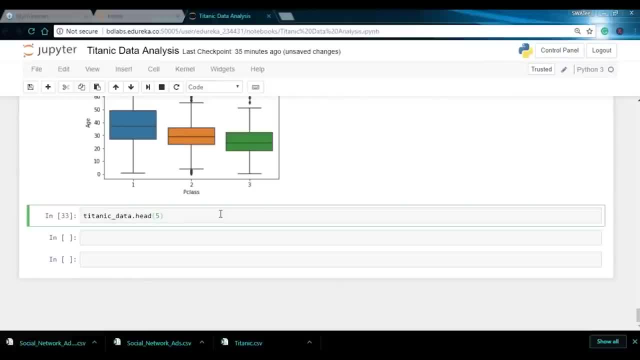 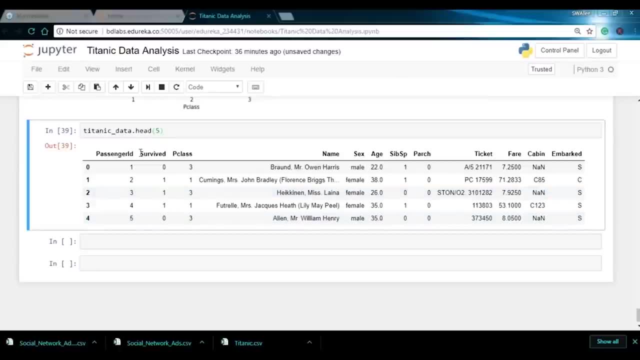 So it's Titanic underscore data. Let's say I just want the five rows. So here we have survived, which is again categorical. So in this particular column I can apply logistic regression. So this can be my Y value or the value that you need to predict. 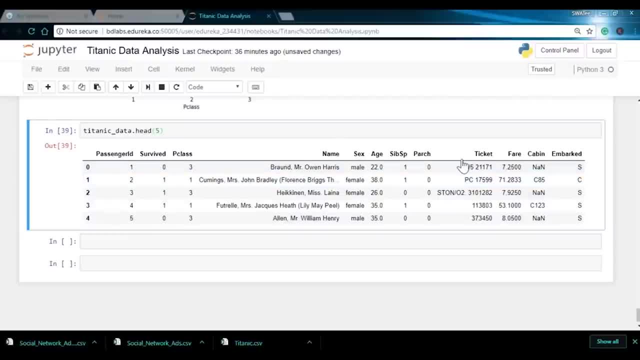 Then we have the passenger class, We have the name, then we have ticket number pair- cabin. So over here we have seen that in cabin we have a lot of null values, or you can say the NAN values is quite visible as well. So first of all we'll just drop this column. 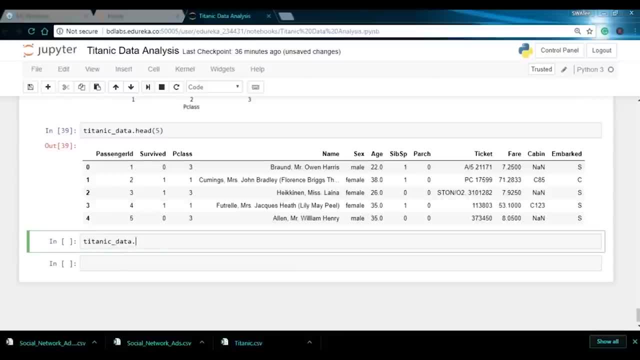 So dropping it, I'll just say Titanic underscore data and I'll simply type and drop and the column which I need to drop- So I have to drop the cabin column- I'll mention the axis equals to one and I'll say: in place also. 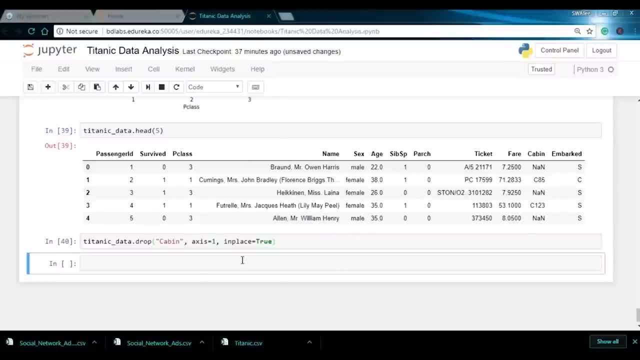 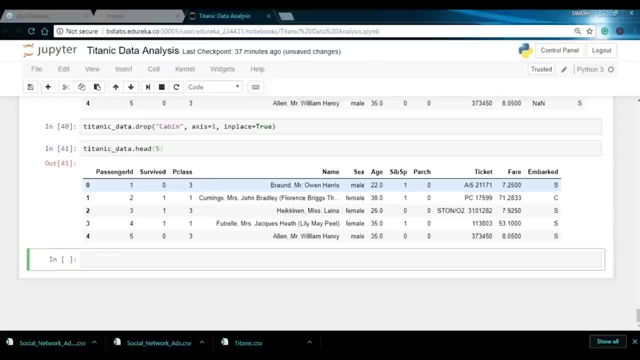 to true. So now again, I'll just print the head and let us see whether this column has been removed from the data set or not. So I'll say Titanic dot head. So as you can see here we don't have cabin column anymore. 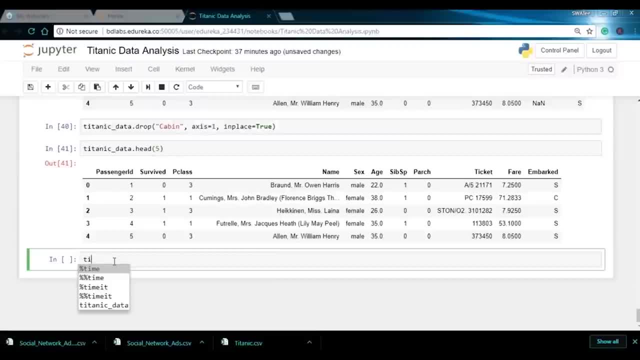 Now you can also drop the NA values. So I'll say: Titanic data dot, drop all the NA values. or you can say NAN, which is not a number, and I'll say: in place is equals to true, It's Titanic. So over here let me again plot the heat map and let's say what. 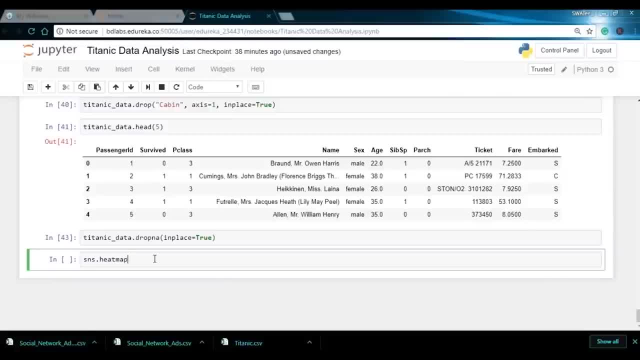 the values which are before showing a lot of null values. has it been removed or not? So I'll say SNS dot heat map. I'll pass in the data set. I'll check it is null. I'll say y tick labels is equals to false. 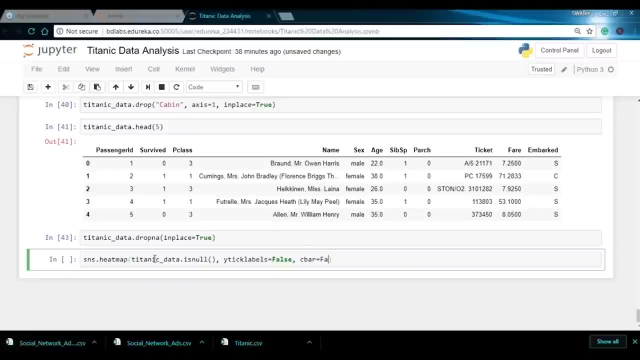 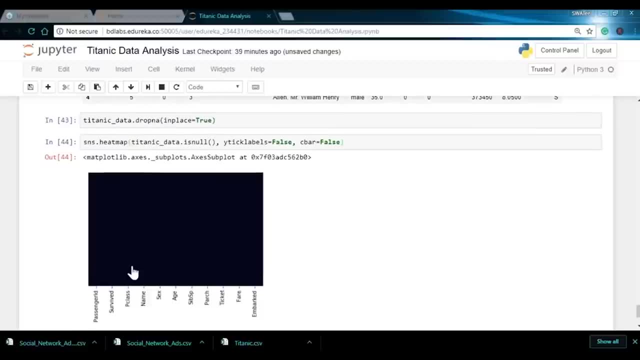 And I don't want color coding, So again I'll say false. So this will basically help me to check whether my values has been removed from the data set or not. So, as you can see here, I don't have any null values. 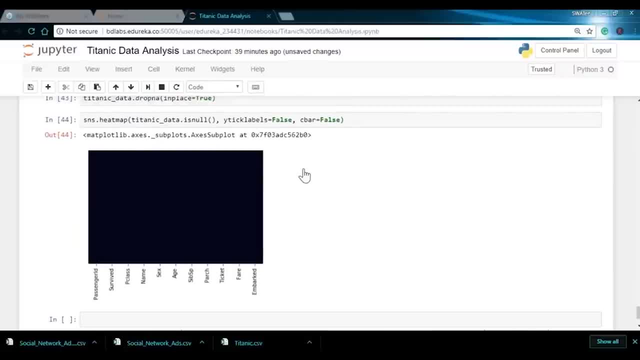 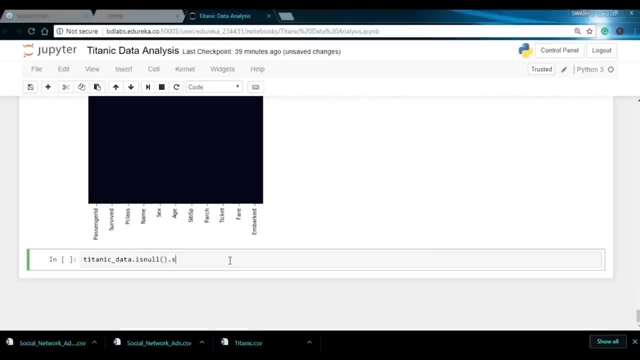 So it's entirely black. now You can actually know the sum as well. So I just go above. So I'll just copy this part and I just use the sum function to calculate the sum. So here that tells me that data set is clean, as in the data set. 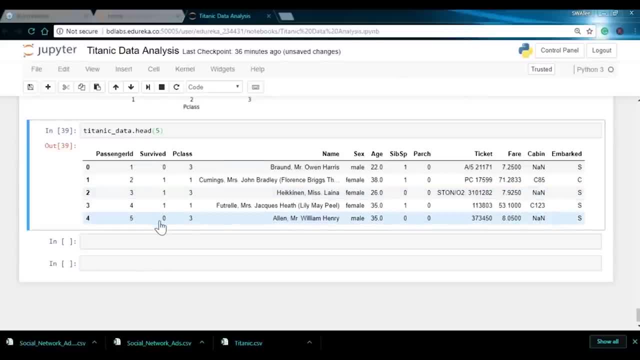 So this can be my Y value or the value that you need to predict. Then we have the passenger class, We have the name, then we have ticket number pair cabin. So over here We have seen that in cabin We have a lot of null values or you can say the nan values is quite visible. 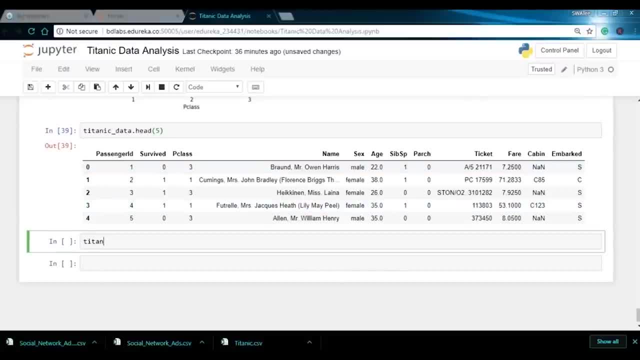 as well. So, first of all, we'll just drop this column. So, dropping it, I'll just say Titanic underscore data and I'll simply type in drop and the column which I need to drop. So I have to drop the cabin column. 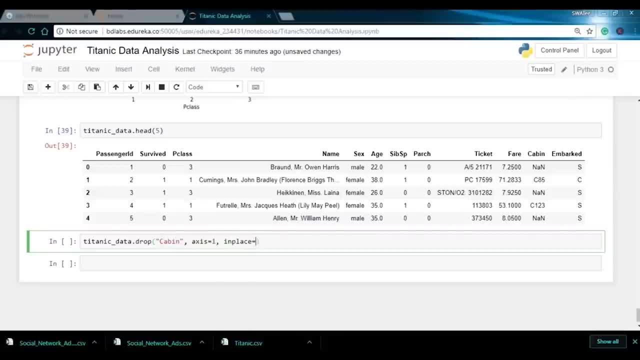 I'll mention the axis equals to 1 and I'll say in place also to true. So now again, I'll just print the head and let us see whether this column has been removed from the data set or not. So I'll say Titanic. 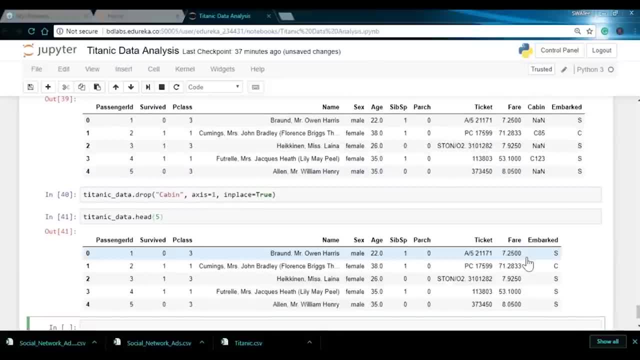 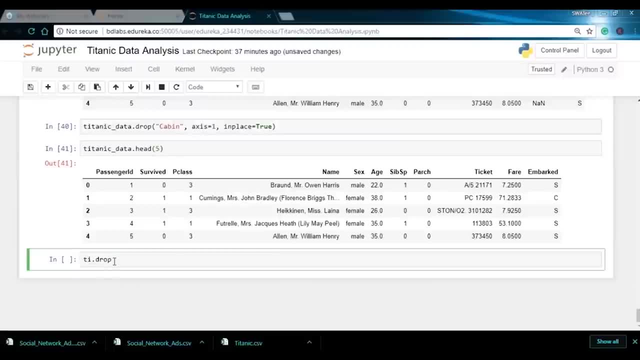 Head. So, as you can see here we don't have cabin column anymore. Now you can also drop the na values. So I'll say Titanic data dot drop all the na values. or you can say nan, which is not a number, and I'll say in place is equals to true. 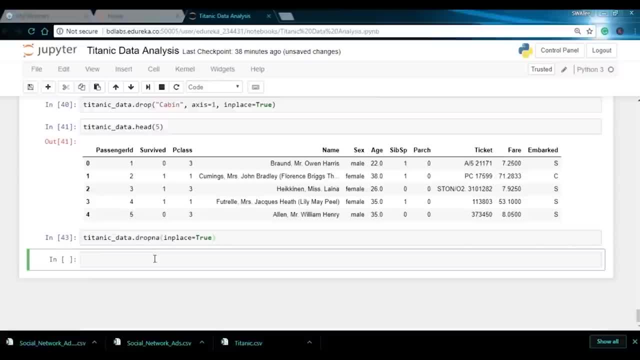 It's Titanic. So over here let me again plot the heat map and let's say what the values which are before showing a lot of null values. has it been removed or not? So I'll say SNS dot heat map, I'll pass in the data set. 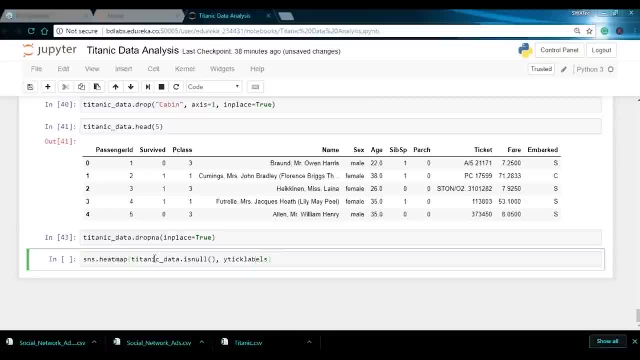 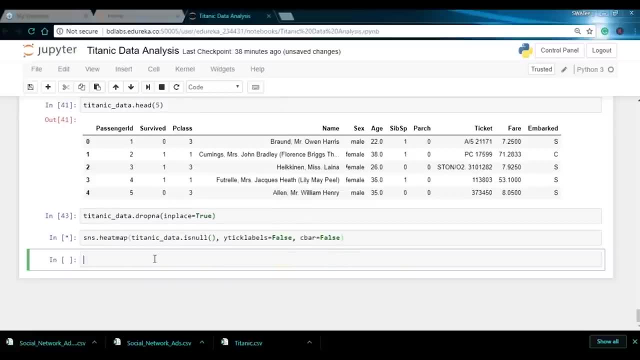 I'll check. it is null, I'll say white tick labels is equals to false And I don't want color coding, So again I'll say false. So this will basically help me to check whether my values has been removed from the data set or not. 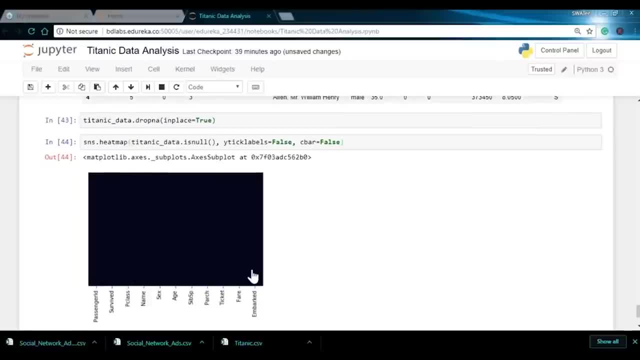 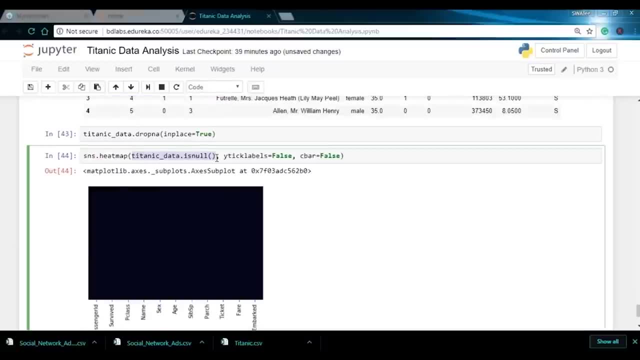 So, as you can see, here I don't have any null values, So it's entirely black. Now you can actually know the sum as well, So I just go above. So I'll just copy this part and I just use the sum function to calculate. 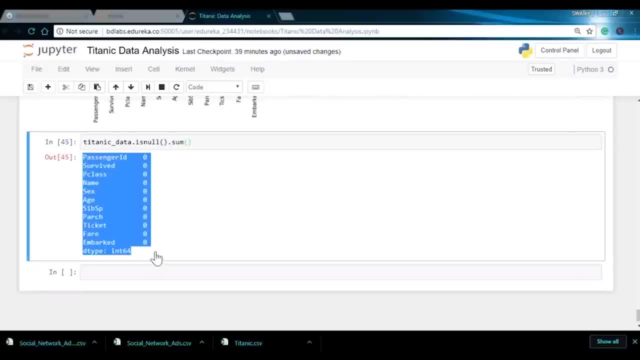 the sum. So here that tells me that data set is clean, as in, the data set does not contain any null value or any any value. So now we have rangled a data. you can say cleaner data. So here we have done just one step in data wrangling, that is, just removing. 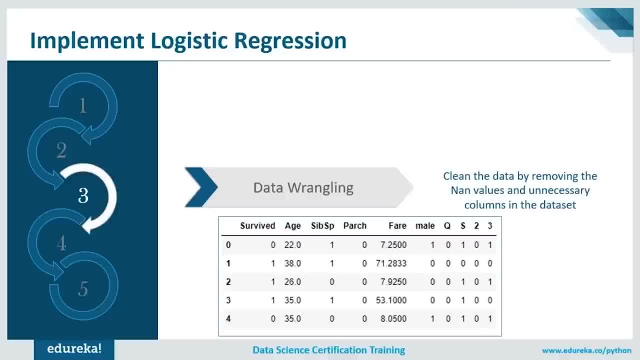 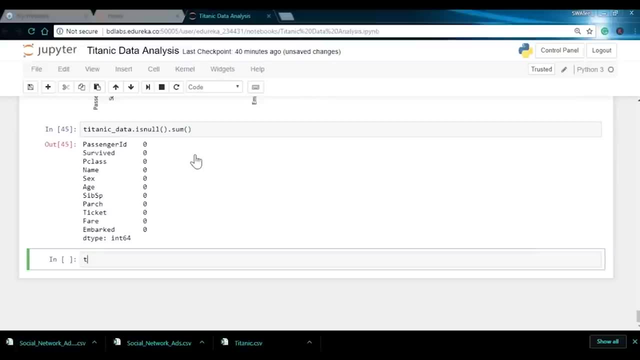 one column out of it. Now you can do a lot of things. you can actually fill in the values with some other values, or you can just calculate the mean and then you can just put in the null values. But now, if I see my data set, so I'll say Titanic data dot head. 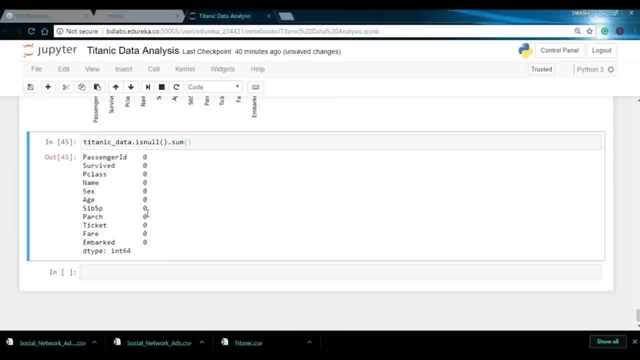 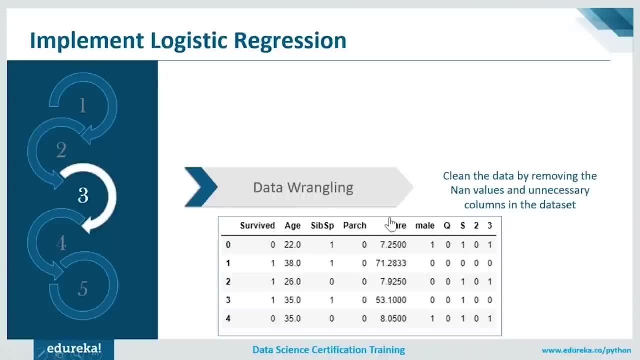 does not contain any null value Or any any n value. So now we have wrangled a data you can say cleaner data. So here we have done just one step in data wrangling, that is, just removing one column out of it. Now you can do a lot of things. 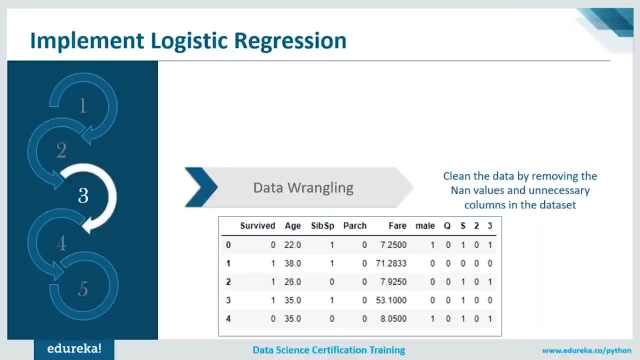 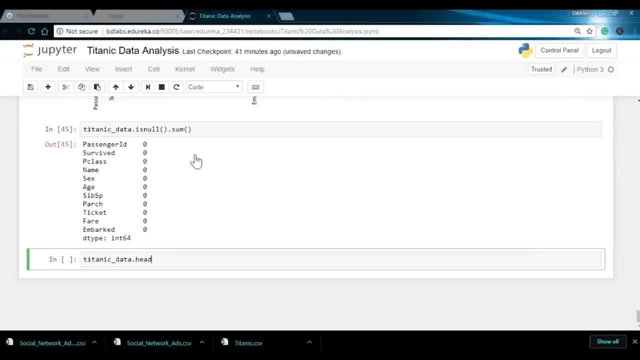 You can actually fill in the values with some other values, or you can just calculate the mean and then you can just put in the null values. But now if I see my data set, so I'll say Titanic data dot head. But now if I see over here, I have a lot of string values. 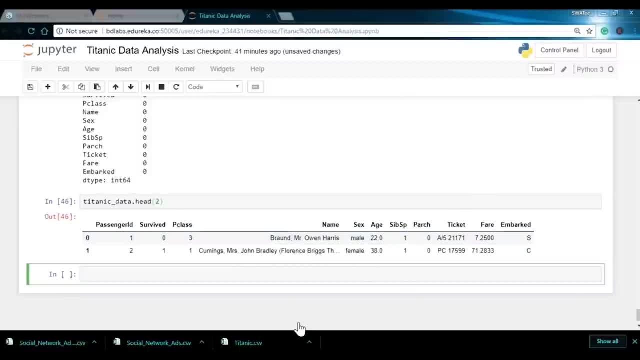 So this has to be converted to categorical variables in order to implement logistic regression. So what we will do, we will convert this to categorical variable into some dummy variables, and this can be done using pandas, because logistic regression just take two values. So whenever you apply machine learning, you need to make sure 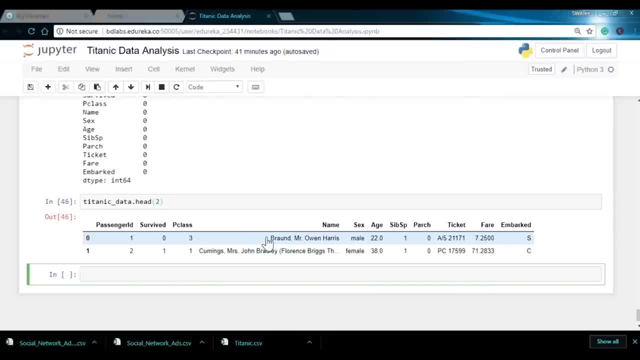 that there are no string values present, because it won't be taking these as your input variables. So using string, you don't have to predict anything. but in my case I have the survive columns, So I need to predict how many people tend to survive and how. 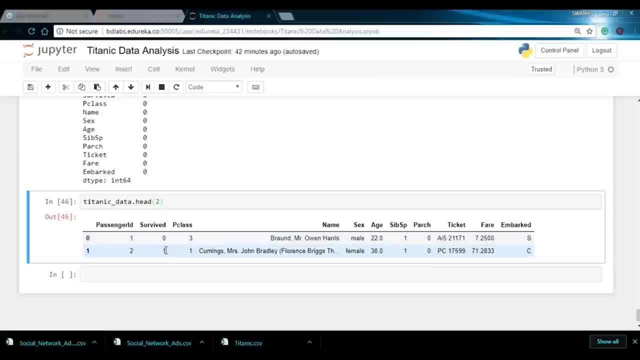 many did not. so zero stands for did not survive and one stands for survive. So now let me just convert these variables into dummy variables. So I'll just use pandas and I'll say: PD dot get dummies. You can simply press tab to auto complete and say: Titanic data. 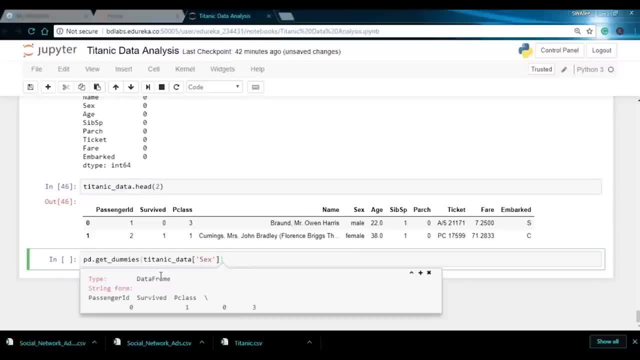 and I'll pass the sex So you can just simply click on ship plus tab to get more information on this. So here we have the type data frame and we have the passenger ID, survived and passenger class. So if you run this you'll see that zero basically stands for. 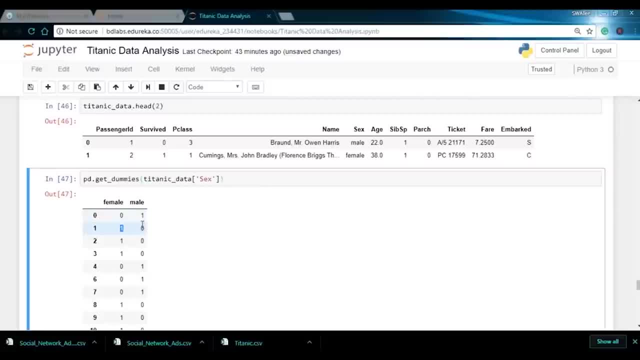 not a female and one stand for it is a female. Similarly for male, zero stands for it's not male and one stand for male. now We don't require both these columns, because one column itself is enough to tell us whether it's male or, you can say, female. 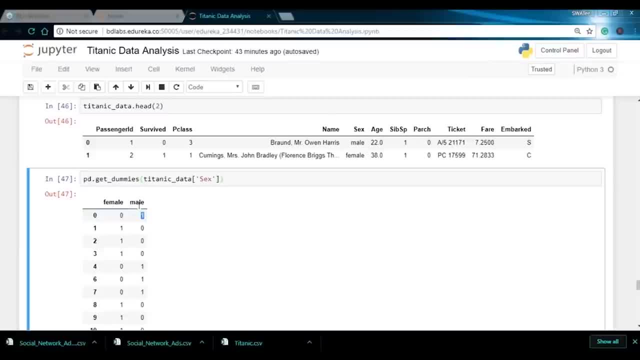 or not. So let's say, if I want to keep only male, I'll say: if the value of male is one, so it is definitely a male and it is not a female. So that is how you don't need both of these values. So for that I just remove the first column. that same female. 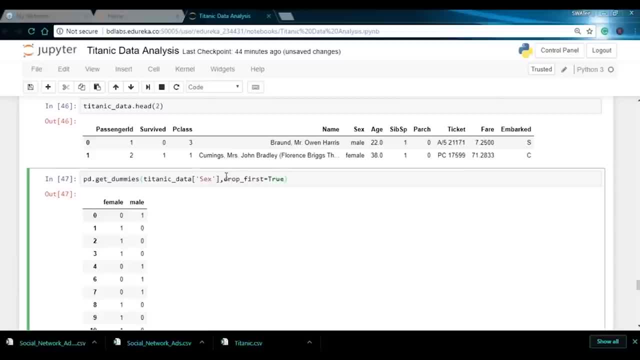 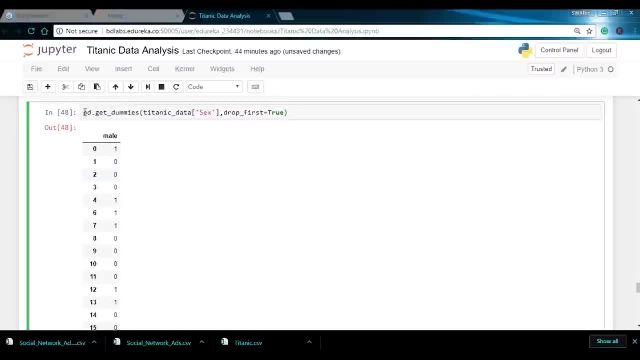 So I'll say drop first and true. So over here it has given me just one column which is male and has the value 0 and 1.. Let me just set this as a variable. It says sex. over here I can say sex dot head. 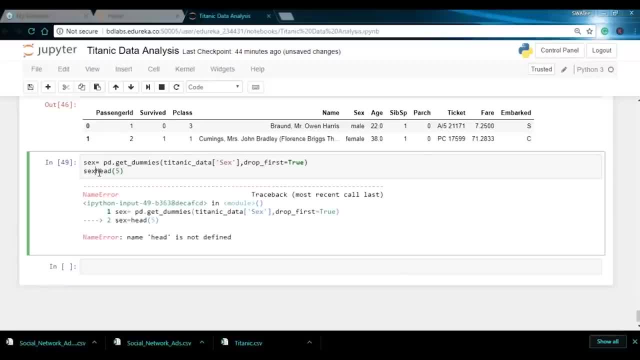 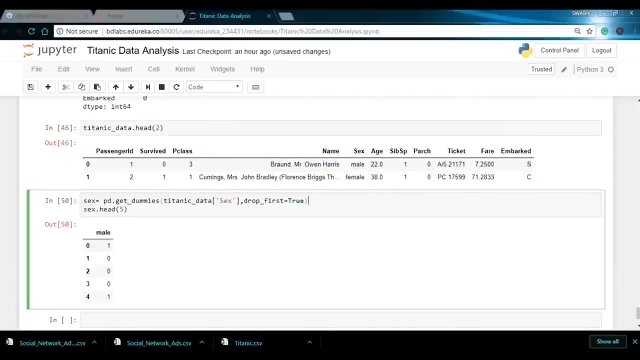 I just want to see the first five rows. Sorry, it's dot, So this is how my data looks like now. here We have done it for sex. Then we have the numerical values in age. We have the numerical values in spouses. 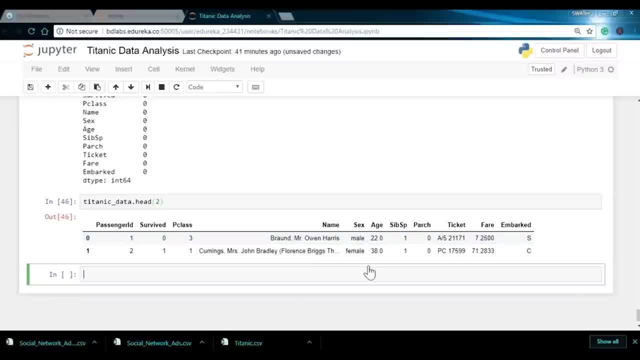 But now, if I see over here, I have a lot of string values, So this has to be converted to categorical variables in order to implement logistic regression. So what we will do, we will convert this to categorical variable into some dummy variables, and this can be done using pandas, because logistic 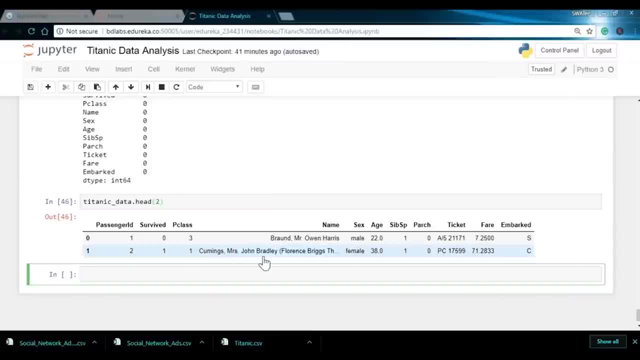 regression just take two values. So whenever you apply machine learning, you need to make sure that there are no string values present, because it won't be taking these as your input variables. So using string, you don't have to predict anything, but in my case I have. 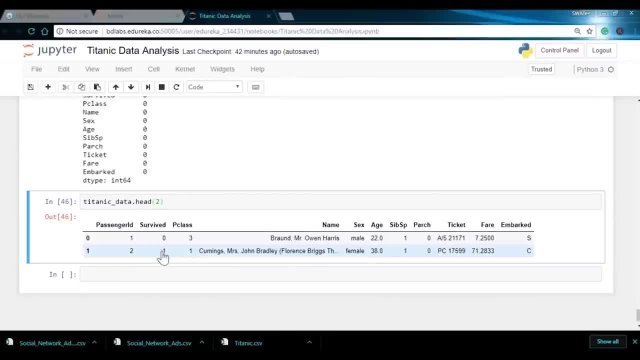 the survive columns. So I need to predict how many people tend to survive and how many did not. so zero stands for did not survive and one stands for survive. So now let me just convert these variables into dummy variables. So I'll just use pandas and I'll say: PD dot get dummies. 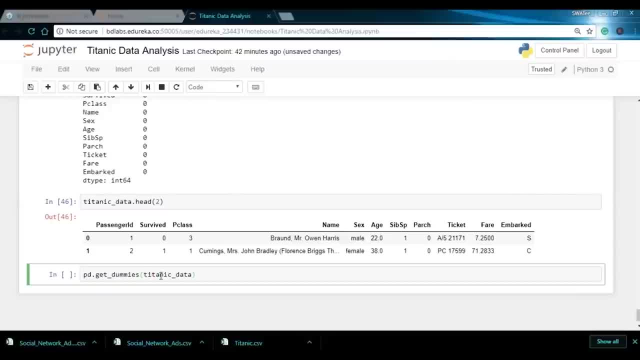 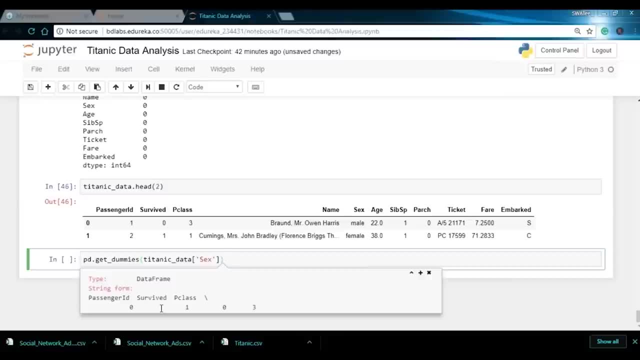 You can simply press tab to autocomplete and say Titanic data and I'll pass the sex. So you can just simply click on ship plus tab to get more information on this. So here we have the type data frame and we have the passenger ID survived and passenger class. 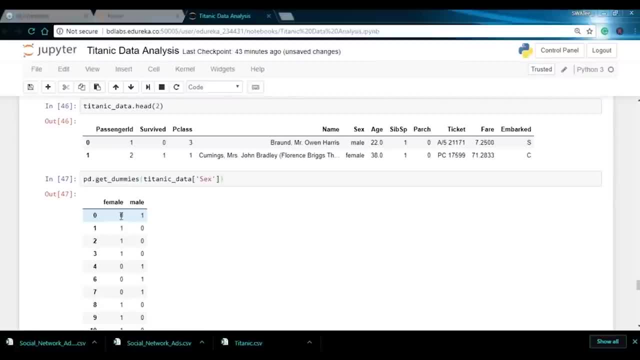 So if you run this, you'll see that 0 basically stands for not a female and one stand for it is a female. similarly, for male: 0 stands for it's not male and one stand for male. Now we don't require both these columns, because one column itself is 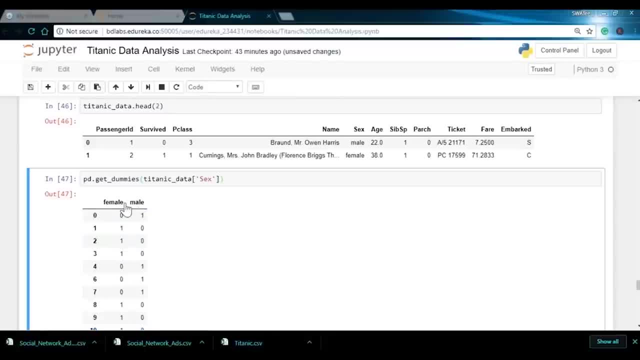 enough to tell us whether it's male, or you can say female or not. So let's say: if I want to keep only male, I'll say: if the value of male is one, so it is definitely a male and it is not a female. So that is how. you don't need both of these values. 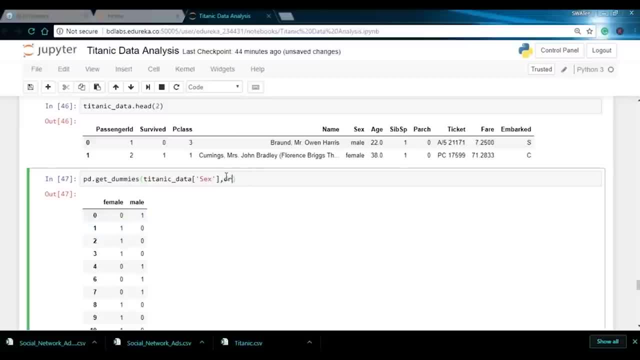 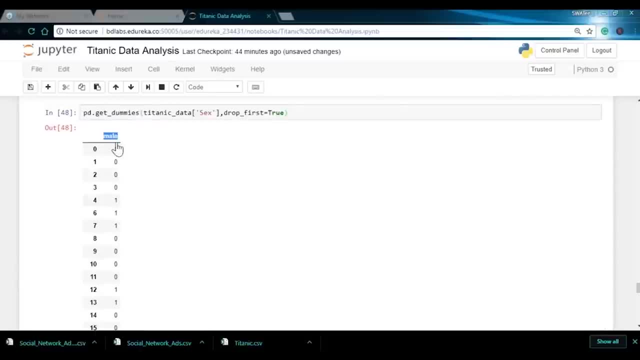 So for that, Let's remove the first column, that same female. So I'll say: drop first, And true. So over here it has given me just one column, which is male and has the value 0 and 1.. Let me just set this as a variable. 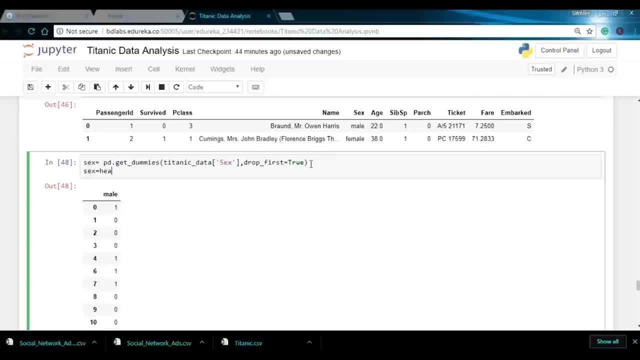 It says sex over here. I can say sex dot head. I just want to see the first five rows. Sorry, it's dot. So this is how my data looks like. Now, here we have done it for sex. Then we have the numerical values in age. 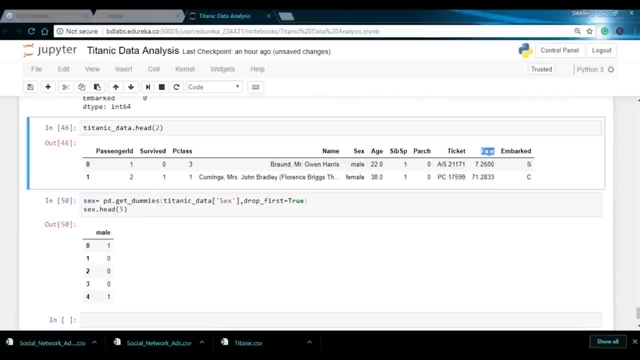 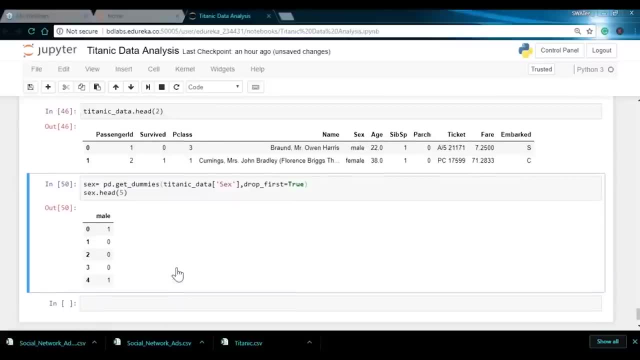 We have the numerical values in spouses, Then we have the ticket number, We have the pair and we have embarked as well. So in embarked the values are in SC and Q. So here also we can apply this get dummy function. So let's say I'll take a variable. 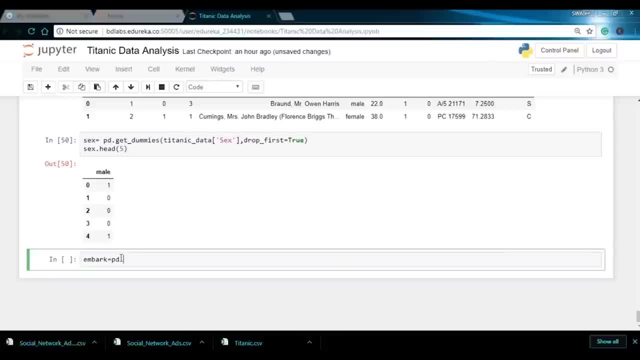 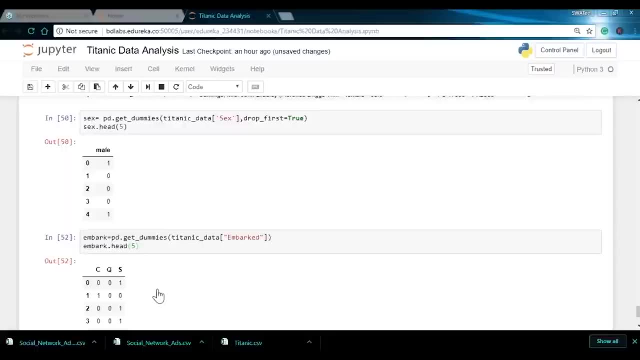 Let's say embark. I'll use the pandas library, I'll enter the column name that is embarked. Let me just print the head of it. So I'll say embarked dot head. So over here we have CQ and S. Now here also we can drop the first column because these two 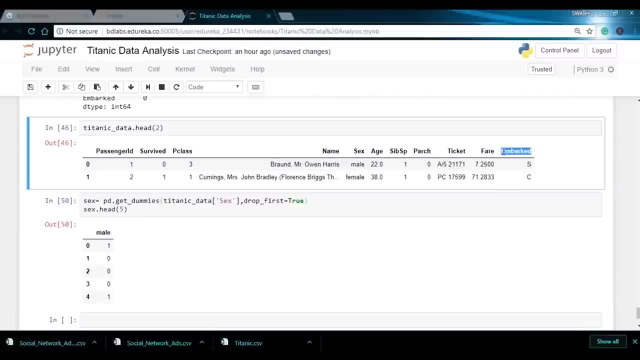 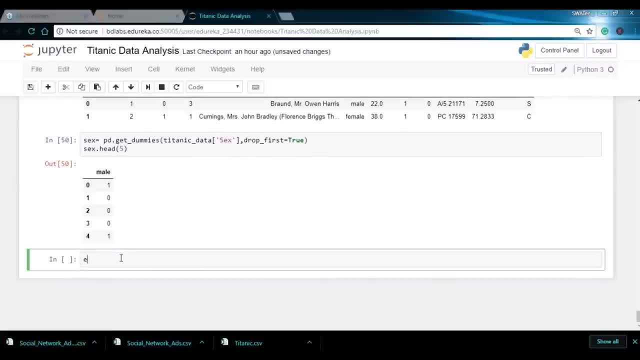 Then we have the ticket number, We have the pair and we have embarked as well. So in embarked the values are in sc And Q. so here also we can apply this get dummy function. So let's say I'll take a variable, Let's say embark. 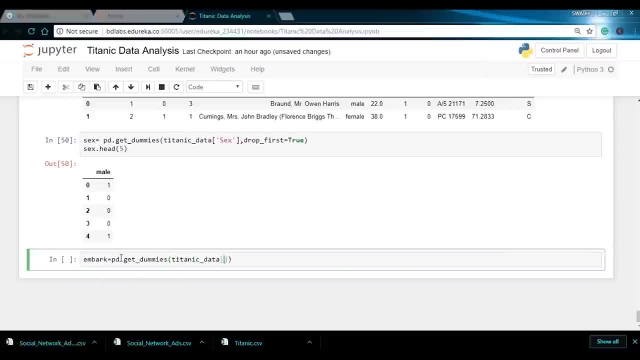 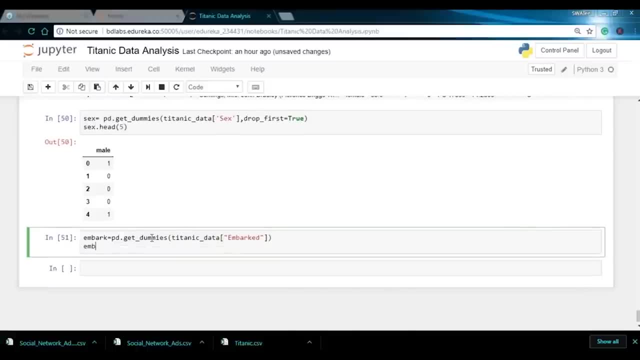 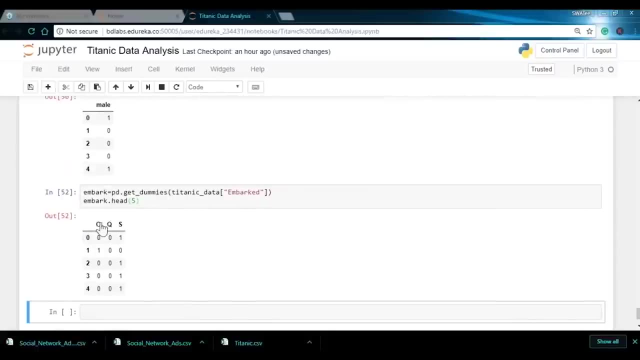 I'll use the pandas library. I'll enter the column name that is embarked. Let me just print the head of it. So I'll say embark dot head. So over here we have CQ and S, now head. also, we can drop the first column because these two values are enough with the passenger. 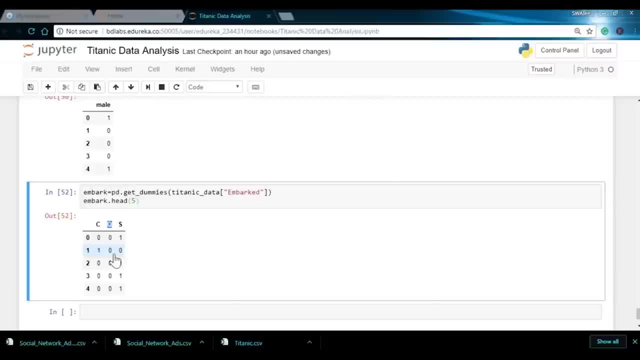 is either traveling for Q, That is, Keenstown S for Southam, and if both the values are zero, then definitely the passenger is from chairbog. That is the third value. So you can again drop the first value. So I'll say drop and true. 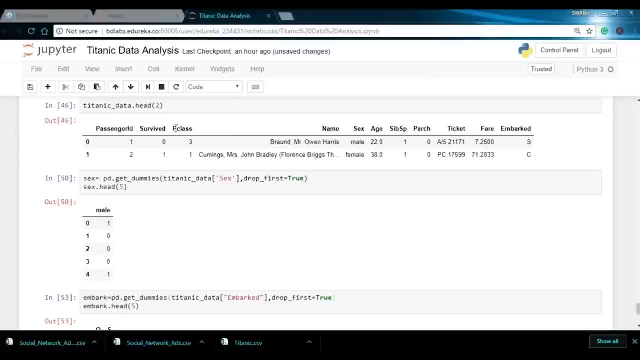 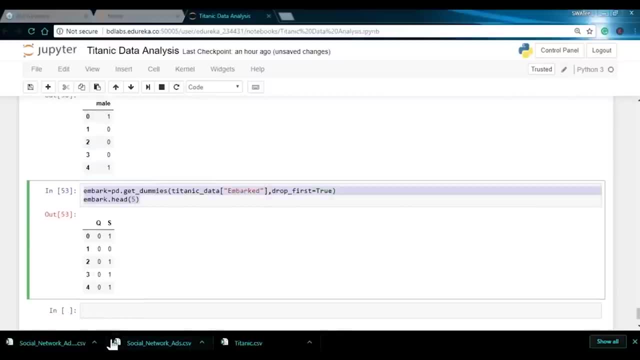 Let me just run this. So this is how my output looks like now. Similarly you can do it for passenger class as well. So here also we have three classes: one, two and three. So I just copy the whole statement. So let's say, I want the variable name. 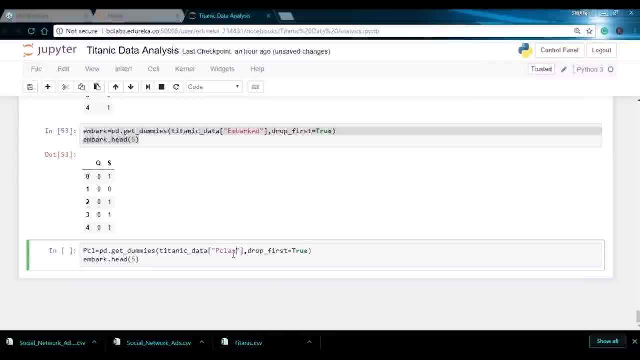 Let's say PCL. I'll pass in the column name, that is P class, and I'll just drop the first column. So here also the values will be one, two or three, and I'll just remove the first column. So here we just left with two and three. 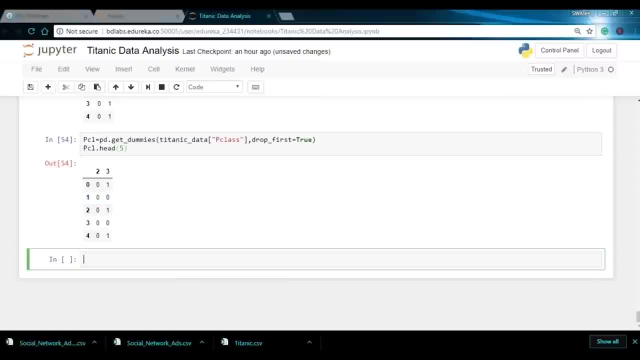 So if both the values are zero, then definitely the passengers traveling in the first class. Now we have made the values as categorical. Now my next step would be to concatenate all these new rows into a data set. I can see Titanic data using the pandas will just concatenate. 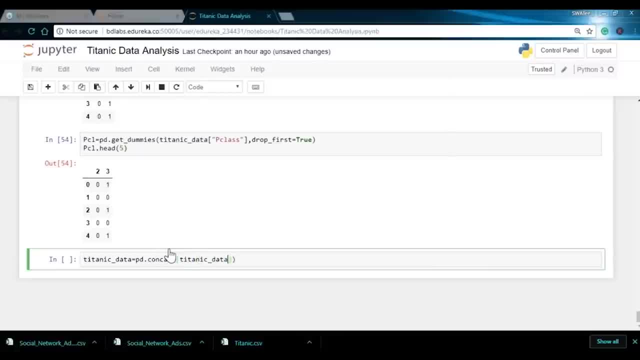 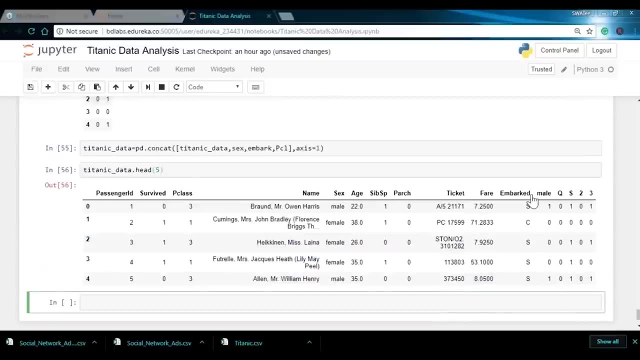 all these columns. So I'll say pcom, cat, And then say we have to concatenate sex, We have to concatenate embark and PCL, and then I'll mention the access to one and just run, this can need to print the head. So over here you can see that these columns have been added. 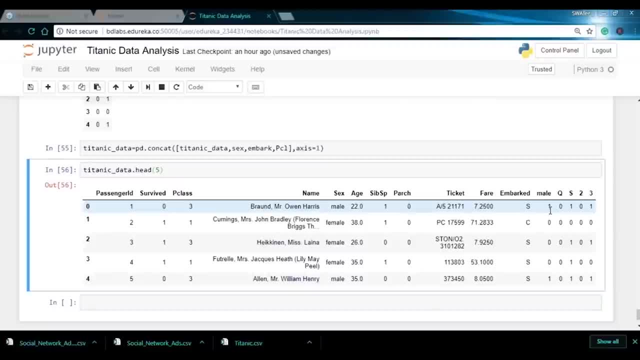 over here. So we have the mail column, which basically tells whether person is male or it's a female. then we have the embark, which is basically Q and S. So if it's traveling from Cunestown, value would be one, else it would be. 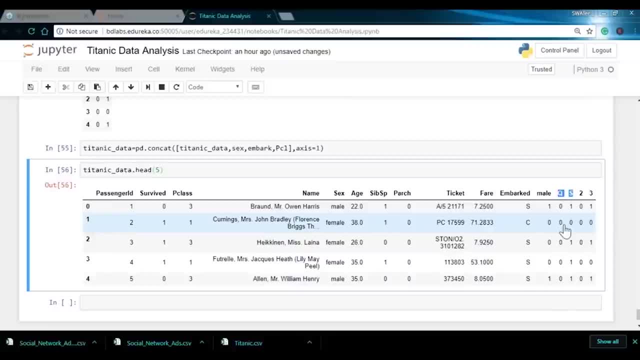 And if both of these values are zero, it is definitely traveling from chair Bob. Then we have the passenger class as two and three. So the value of both these is zero. then the passengers traveling in class one. So I hope you got this till now. 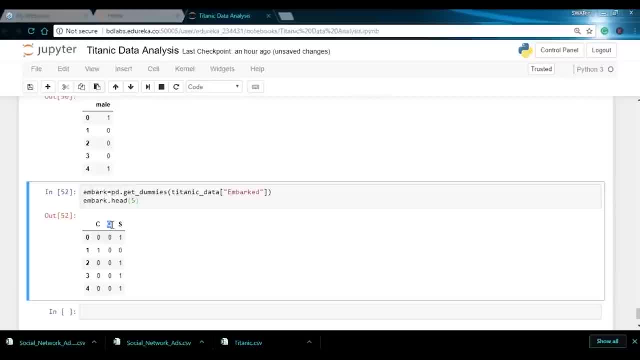 values are enough with. the passenger is either traveling for Q, that is, Kuenstown S for Southampton, and if both the values are 0, then definitely the passenger is from Cherbourg. That is the third value, So you can again drop the first value. 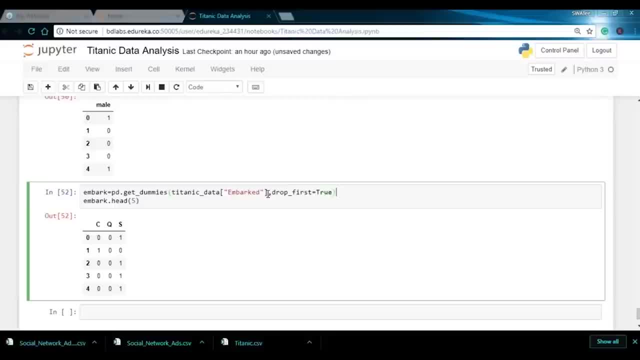 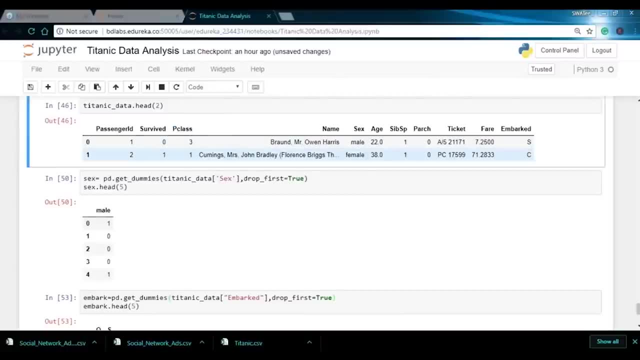 So I'll say drop and true, Let me just run this. So this is how my output looks like now. Similarly, you can do it for passenger class as well. So here also we have three classes: one, two and three. So I'll just copy the whole statement. 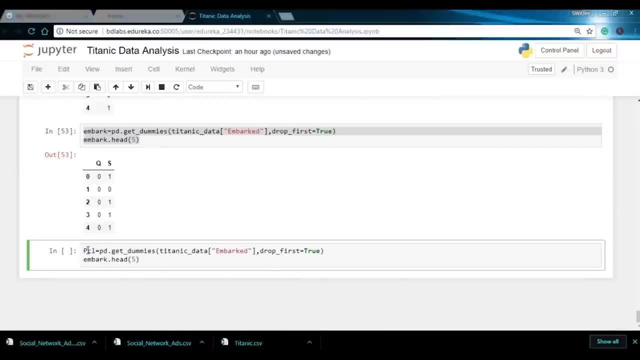 So let's say I want the variable name, Let's say PCL. I'll pass in the column name, that is P class, and I'll just drop the first column. So here also the values will be 1, 2 or 3, and I'll just remove the. 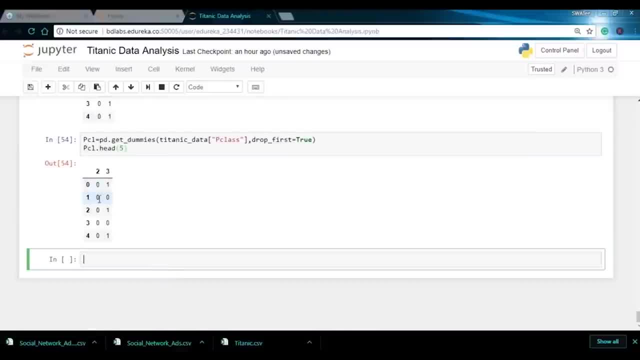 first column. So here we just left with 2 and 3.. So if both the values are 0, then definitely the passengers traveling in the first class. Now we have made the values as categorical. Now my next step would be to concatenate all these new rows. 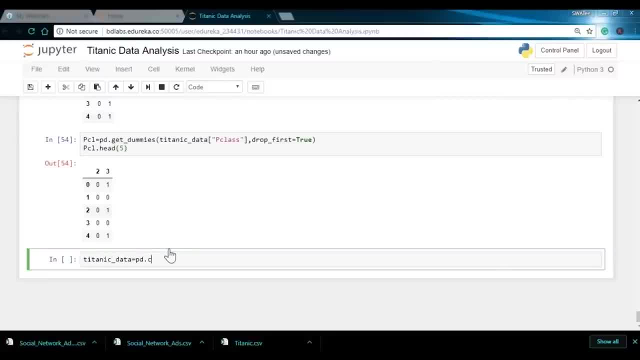 into a data set. or you can say Titanic data using the pandas will just concatenate all these columns. So I'll say pconcat and I'll say we have to concatenate sex, We have to concatenate mbav and PCL, and then I'll mention the. 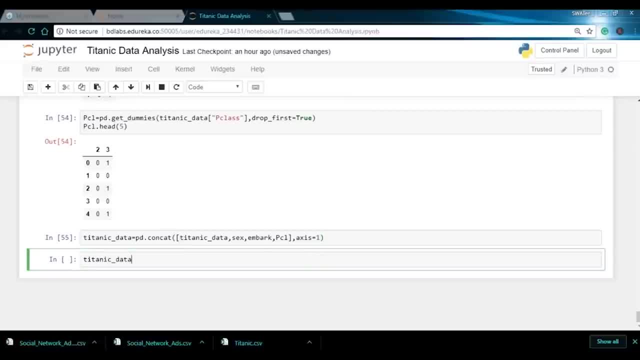 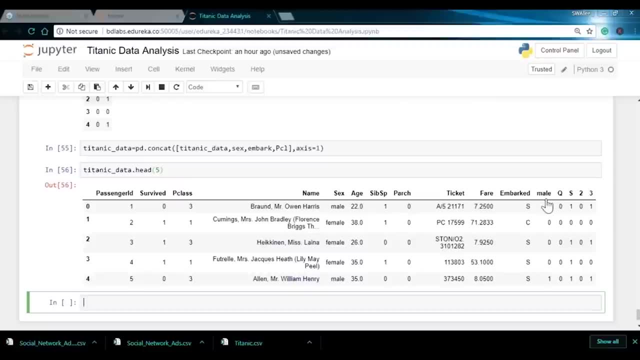 access to one and just run this. I need to print the head, So over here you can see that these columns have been added over here. So we have the male column with: Basically tells whether a person is male or it's a female. then 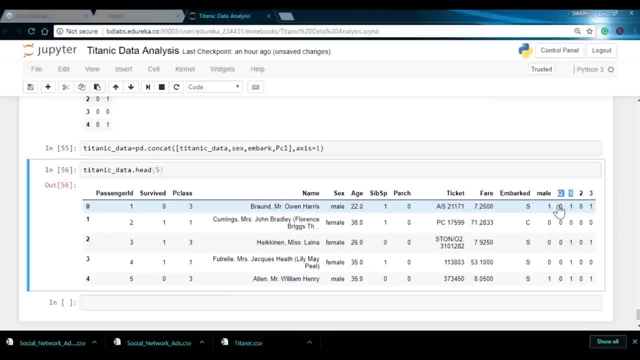 we have the embark, which is basically Q and S. So if it's traveling from Cunestown, value would be 1, else it would be 0, and if both of these values are 0, it is definitely traveling from chair Bob. Then we have the passenger class as 2 and 3.. 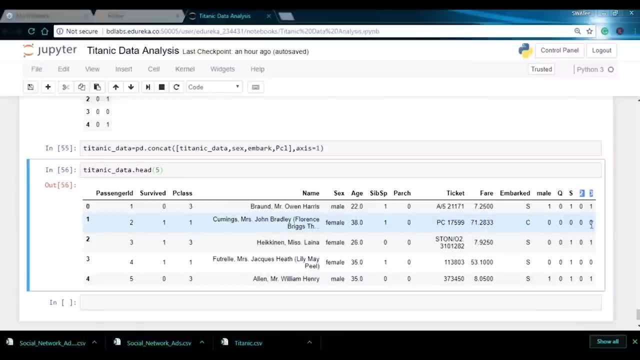 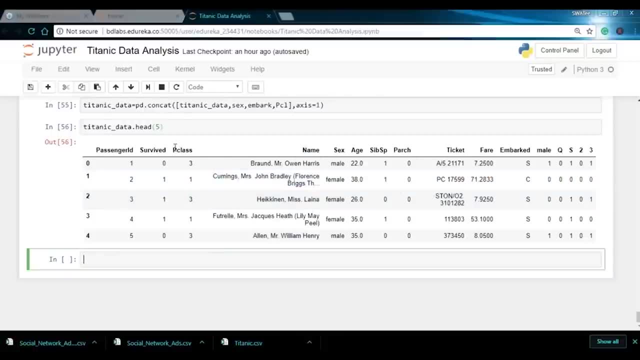 So the value of both these is 0, then the passengers traveling in class 1.. So I hope you got this till now. Now, These are the irrelevant columns that we have it over here, So we can just drop. these columns will dropping. 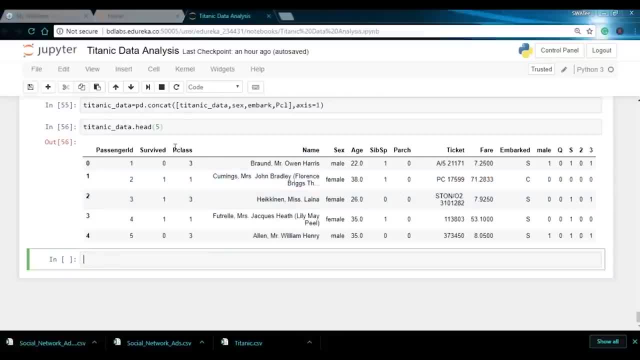 Now These are the irrelevant columns that we have it over here, So we can just drop these columns. will dropping P class, the embarked column and the sex column. So I just type in Titanic data dot drop and mention the columns that I want to drop. 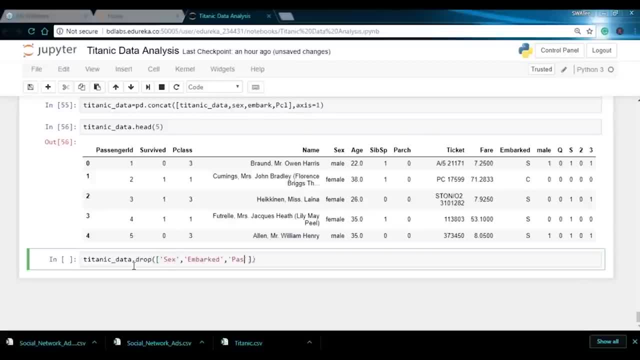 So I'll say I even delete the passenger ID, because it's nothing but just the index value which is starting from one, So I'll drop this as well. Then I don't want name as well, So I'll delete name as well. 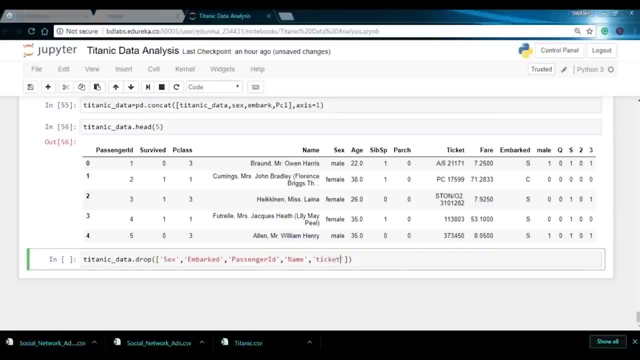 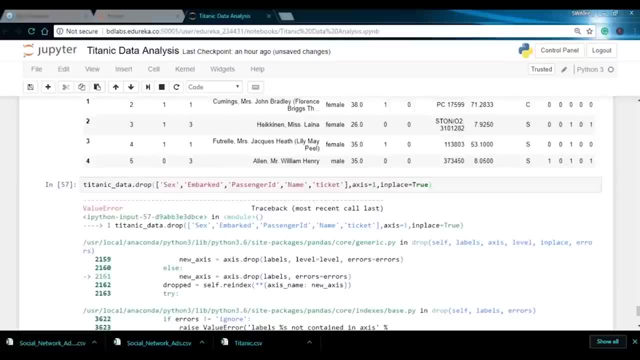 Then what else we can drop. we can drop the ticket as well, And then I just mentioned the access, and I'll say: in place is equals to true. Okay, so my column name starts Uppercase, So these has been dropped now. 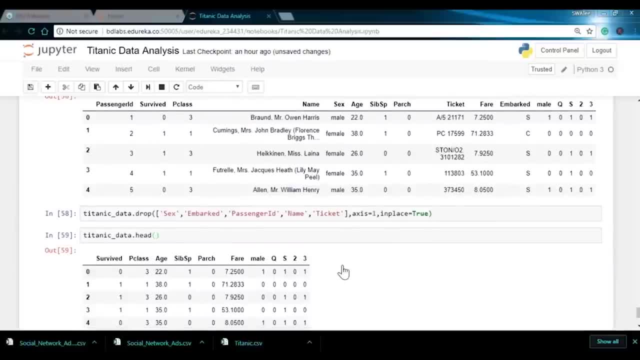 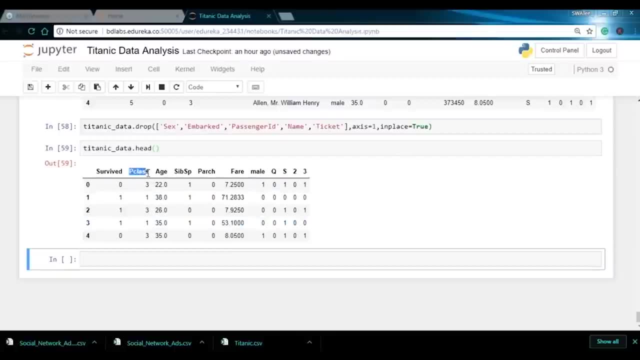 Let me just print my data set again. So this is my final data set, guys. We have the survived column, which has the value 0 and 1. then we have the passenger class, or we forgot to drop this as well, So no worries. 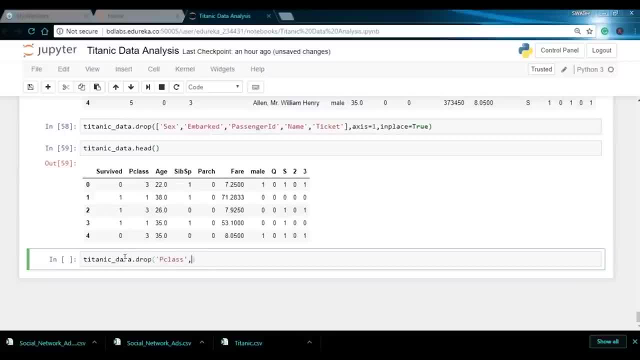 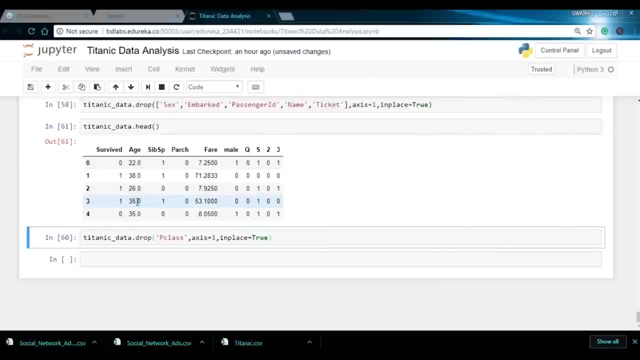 I'll drop this again. So now let me just run this. So over here, we have the survive, We have the age, We have the Sib SP, We have the part, We have fair meal, And these we have just converted. 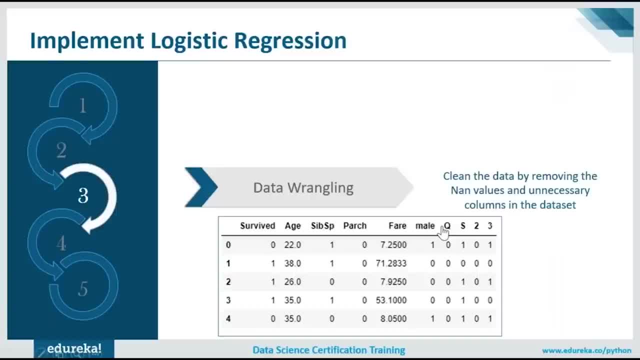 So here we have just performed data wrangling, or you can say clean the data, and then we have just converted the values of gender to male, then embarked to Q and S and the passenger class to 2 and 3.. So this was all about my data wrangling. 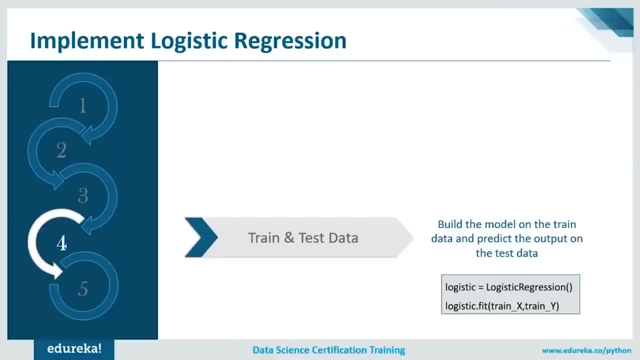 or just cleaning the data. Then my next step is training and testing your data. So here we will split the data set into train subset and test subset, and then what we'll do will build a model on the train data and then predict the output on your test. 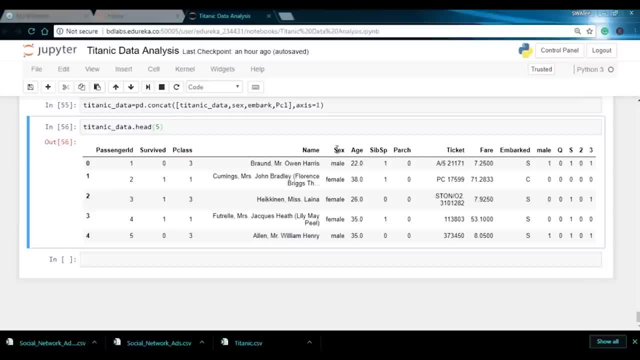 P class, the embarked column and the sex column. So I just type in Titanic data dot drop and mention the columns that I want to drop. So I'll say I even delete the passenger ID because it's nothing but just the index value which is starting from one. 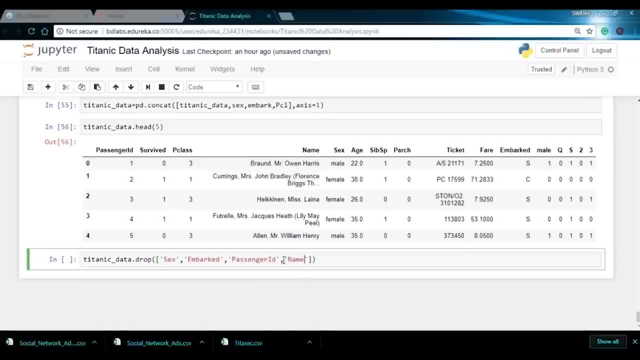 So I'll drop this as well. Then I don't want name as well, So I'll delete name as well. Then what else we can drop? we can drop the ticket as well, And then I just mentioned the axis and I'll say: in place is 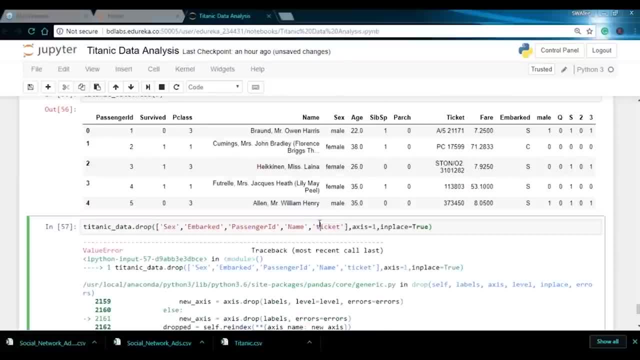 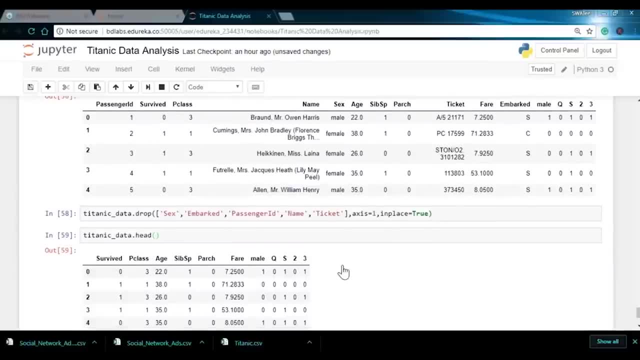 equals to true. Okay, so my column name starts from uppercase, So these has been dropped. now Let me just print my data set again. So this is my final data set, guys. We have the survived column, which has the value 0 and 1. then 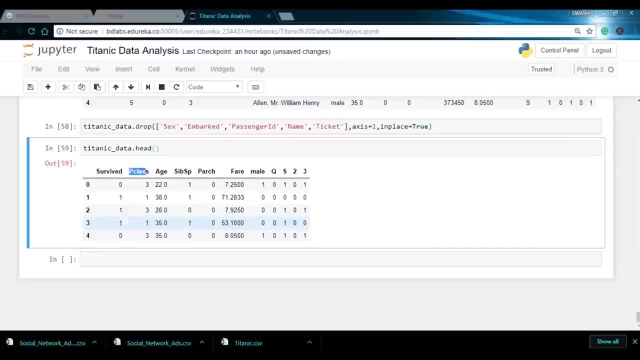 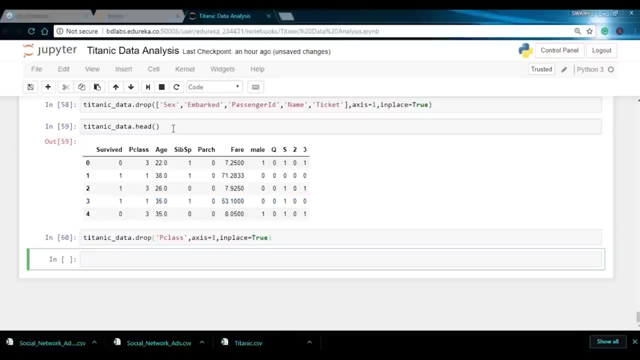 we have the passenger class, or we forgot to drop this as well. So no worries, I'll drop this again. So now let me just run this Over here. We have the survive, We have the age, We have the Sib SP. 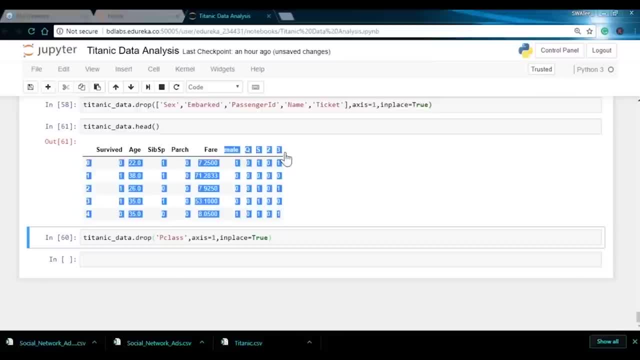 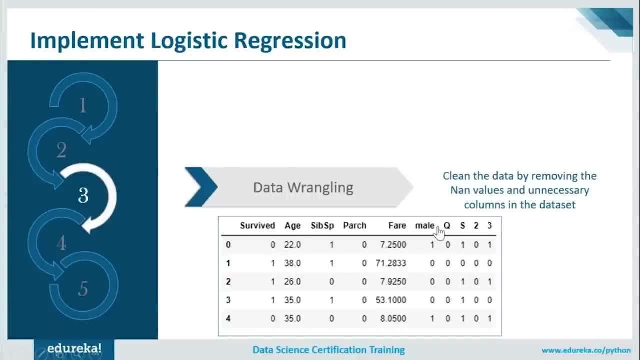 We have the parts, We have fair meal, and these we have just converted. So here we have just performed data wrangling, or you can say clean the data, and then we have just converted the values of gender to male, then embarked to Q and S and the passenger class. 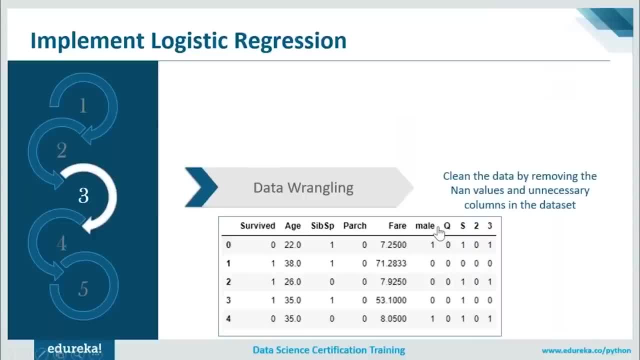 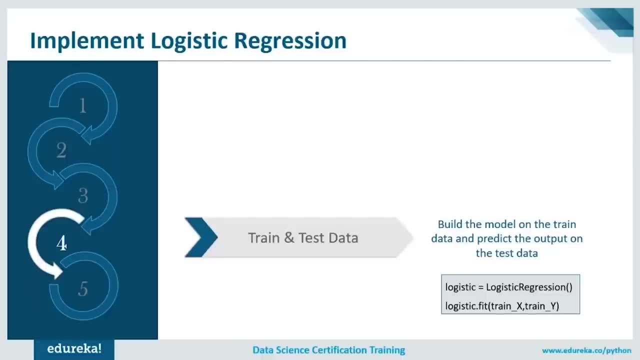 to 2 and 3.. So this was all about my data wrangling, or just cleaning the data. Then my next step is training and testing your data. So here We will split the data set into train subset and test subset, and then what we'll do will build a model on the train data. 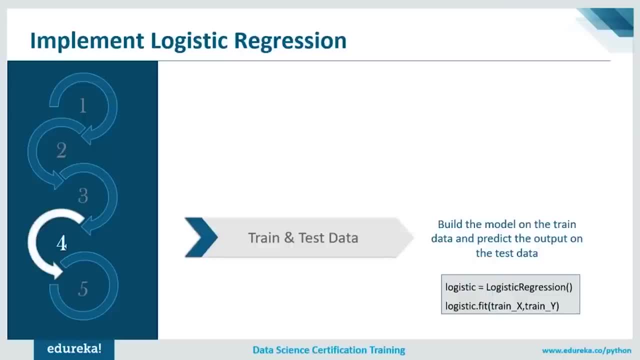 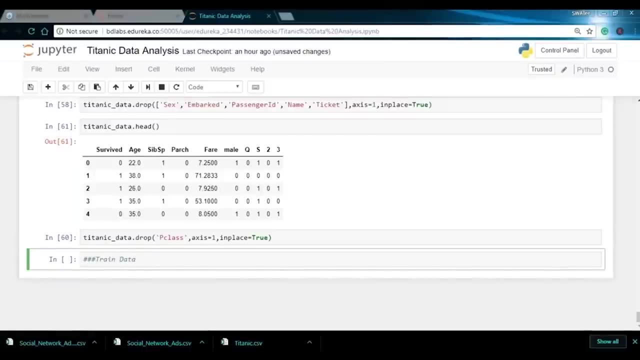 and then predict the output on your test data set. So let me just go back to Jupiter and let us implement this as well. over here, I need to train my data set, So I'll just put this in the heading 3.. So, over here, you need to define your dependent variable and 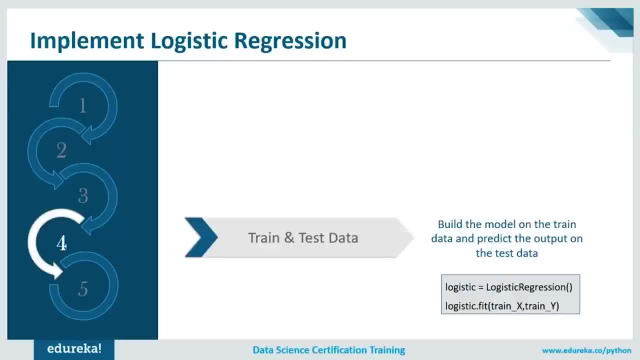 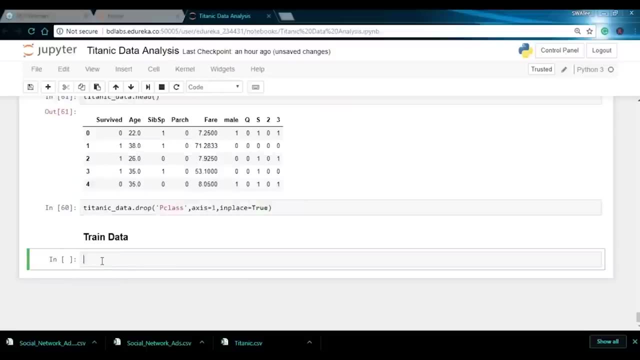 data set. So let me Just go back to Jupiter and let us implement this as well. Over here, I need to train my data set, So I'll just put this in the heading 3.. So over here, you need to define your dependent variable. 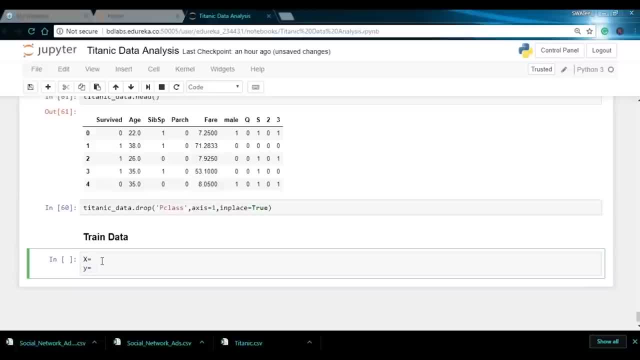 and independent variable. So here my Y is the output. I can say the value that I need to predict. over here I'll write Titanic data, I'll take the column which is survive. So basically I have to predict this column, whether the passenger 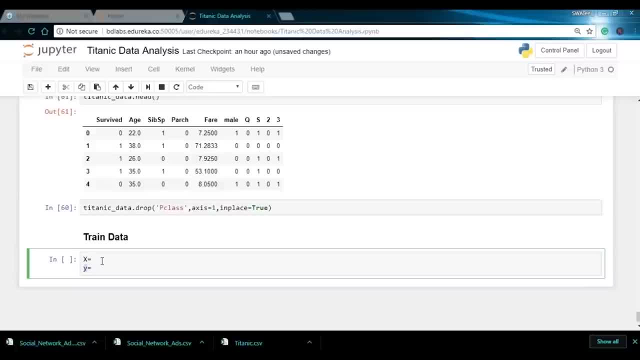 independent variable. So here my Y is the output or you can say the value that I need to predict. over here I'll write Titanic Data, I'll take the column which is survive. So basically I have to predict this column, whether the passenger survived or not, and, as you can see, we have the discrete outcome. 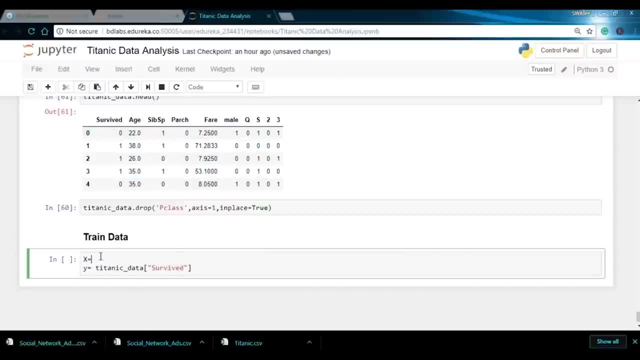 which is in the form of 0 and 1 and rest all the things. we can take it as a features or you can say independent variable. So I'll say: Titanic data not drop. So we'll just simply drop the survive and all the other columns. 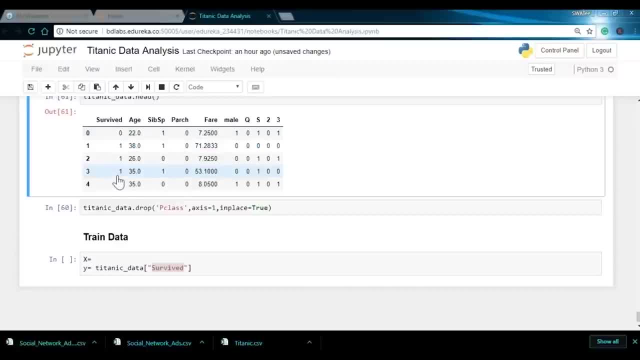 survived or not and, as you can see, we have the discrete outcome, which is in the form of 0 and 1 and rest all the things. we can take it as a features or you can say independent variable. So I'll say Titanic data, not drop. 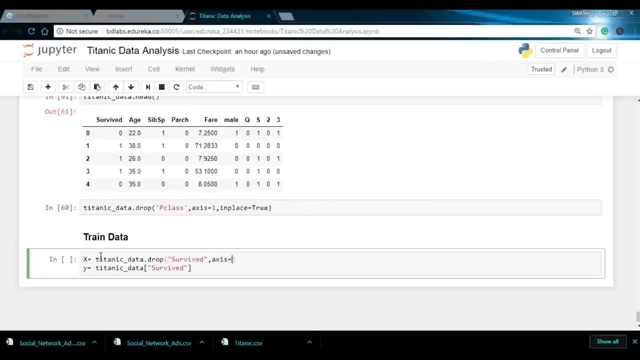 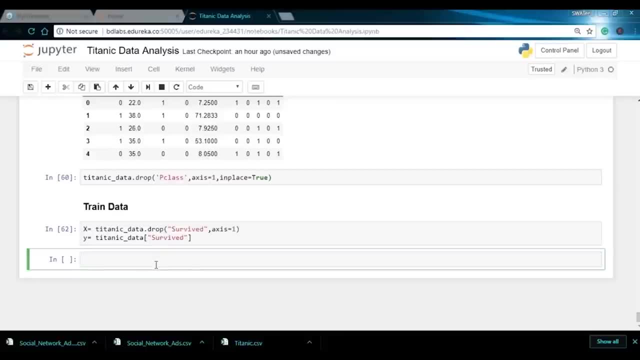 So we'll just simply drop the survive and all the other columns will be my independent variable. So everything else are the features which leads to the survival rate. So, once we have defined the independent variable and the dependent variable, next step is to split your data. 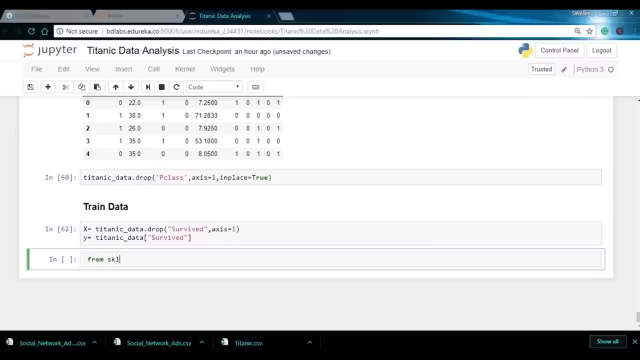 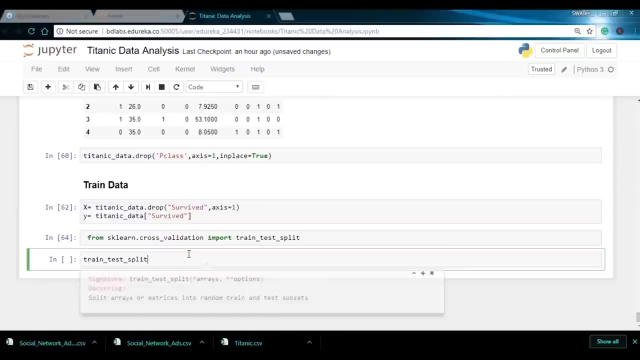 into training and testing subset. So for that we'll be using sklearn. I just type in from sklearn dot: cross validation: Import train test plate. Now here, if you just click on shift and tab you can go to the documentation and you can just see the examples over here. 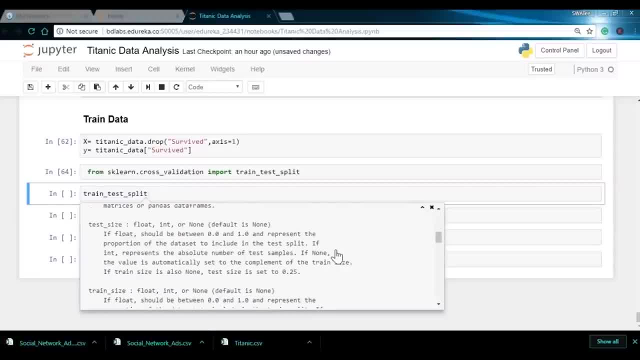 I'll click on plus to open it and then I just go to examples and see how you can split your data. So over here you have X train, X test, Y train, Y test and then, using this train test plate, You can just pass in your independent variable and dependent variable. 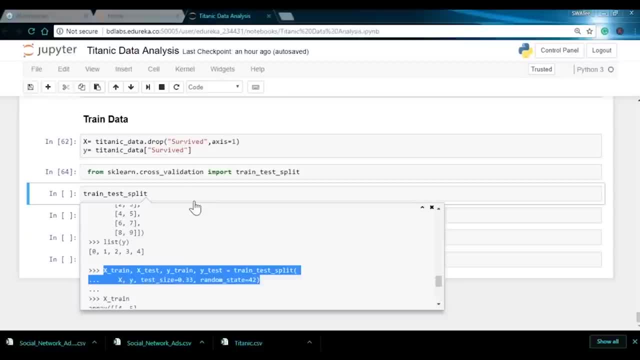 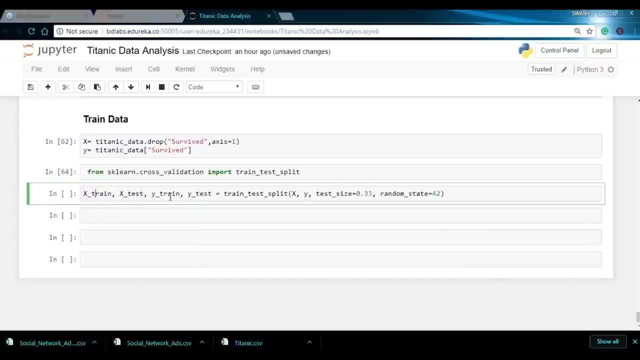 and just define a size and a random state to it. So let me just copy this and I'll just paste it over here. Over here will train test. then we have the dependent variable train and test and using the split function will pass in the independent. 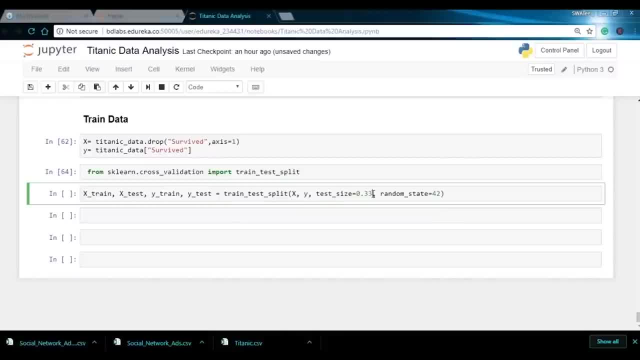 and dependent variable, and then we'll set a split size. So let's say I'll put it at 0.3.. So this basically means that your data set is divided in 0.3, that is, in 70-30 ratio, and then I can add any random state. 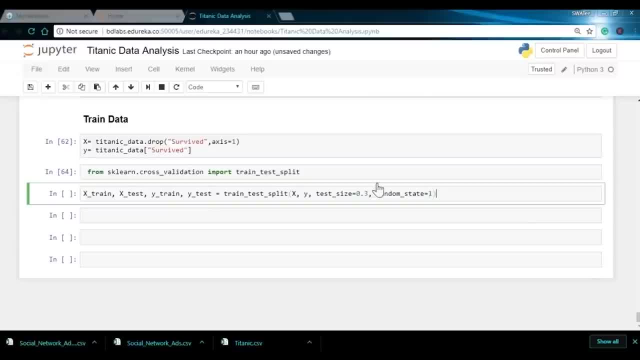 So let's say I'm applying one. This is not necessary. If you want the same result as that of mine, you can add the random state. So this will basically take exactly the same sample every time. Next, I have to train and predict by creating a model. 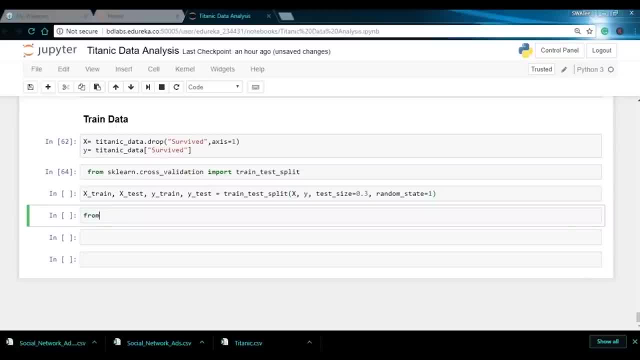 So here logistic regression will grab from the linear regression. So next I'll just type in: from sklearn dot linear model, Import logistic regression. Next I'll just create the instance of this logistic regression model. So I'll say logistic regression model. Log model is equals to logistic regression. 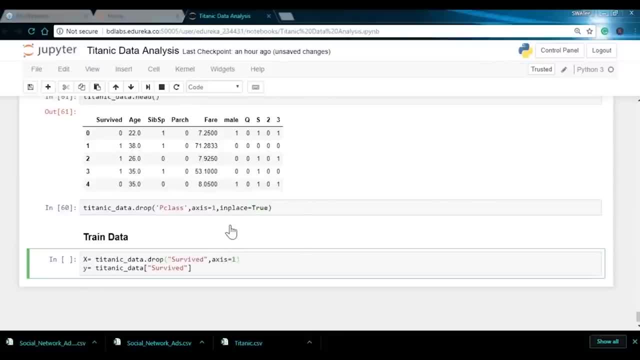 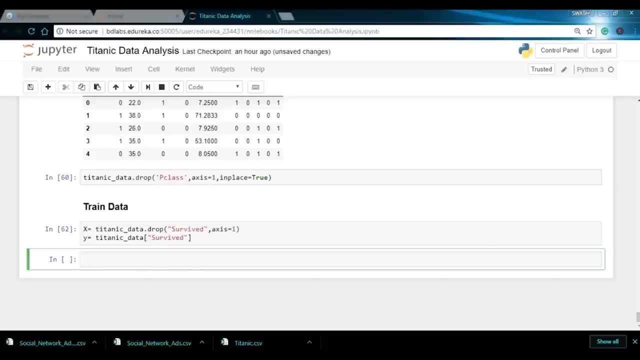 will be my independent variable. So everything else are the features which leads to the survival rate. So once we have defined the independent variable and the dependent variable, next step is to split your data into training and testing subset. So for that we'll be using sklearn. I just type in from sklearn: 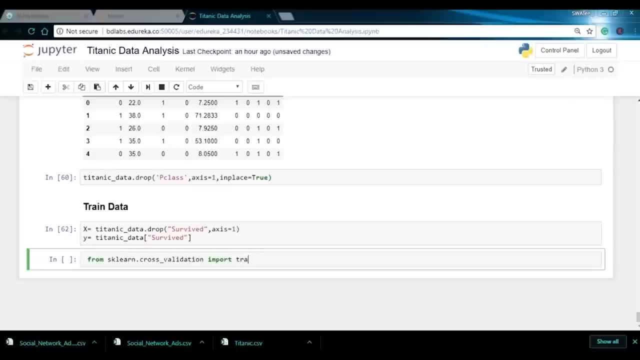 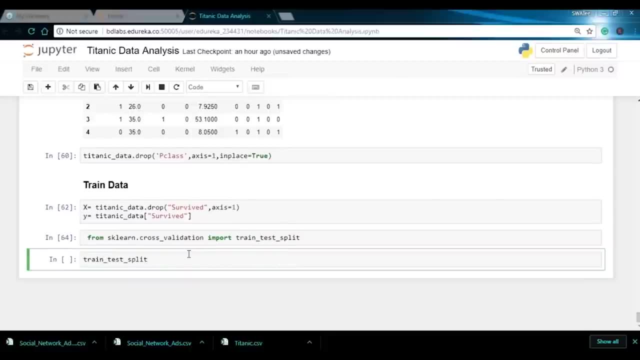 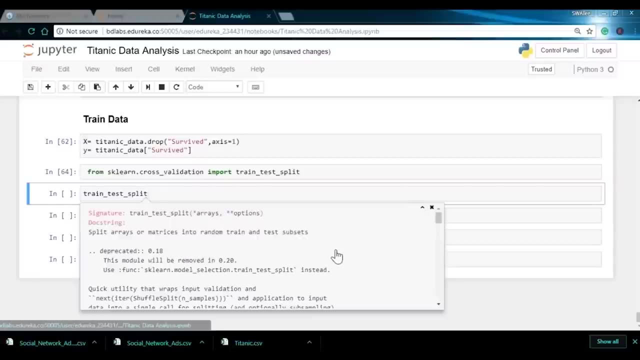 dot cross validation- Import train test plate. Now here: if you just click on shift and tab, you can go to the documentation and you can just see the examples over here. I'll click on plus to open it And then I just go to examples and see how you can split your. 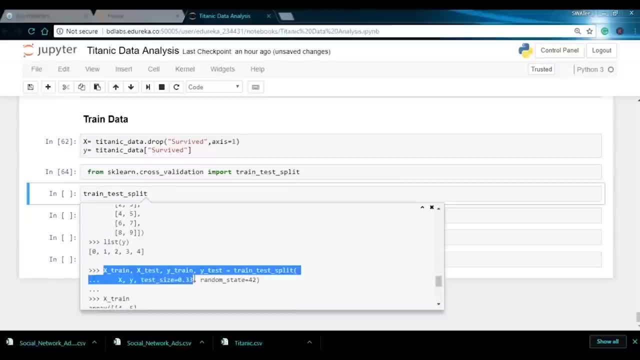 data. So over here you have X train, X test, Y train, Y test and then using this train test plate, You can just pass in your independent variable and dependent variable and just define a size and a random state to it. So let me just copy this and I'll just paste it over here. 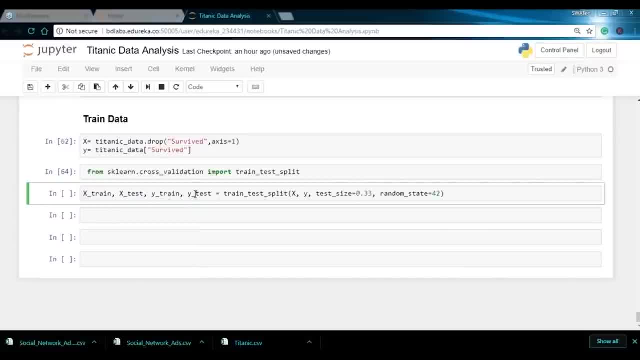 Over here will train test. Then we have the dependent variable- train and test- and using the split function will pass in the independent and dependent variable And then we'll set a split size. So let's say I'll put it at 0.3.. 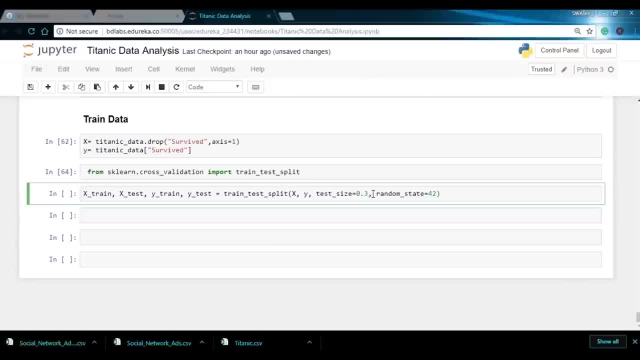 So this basically means that your data set is divided in 0.3, that is, in 70-30 ratio, and then I can add any random state to it. So let's say I'm applying one. This is not necessary. If you want the same result as that of mine, you can add the. 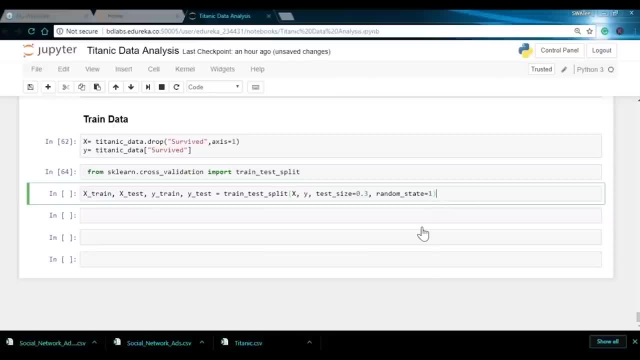 random state. So this will basically take exactly the same sample every time. next I have to train and predict by creating a model. So here logistic regression will grab from the linear regression. So next I'll just type in from sklearn dot. linear model. 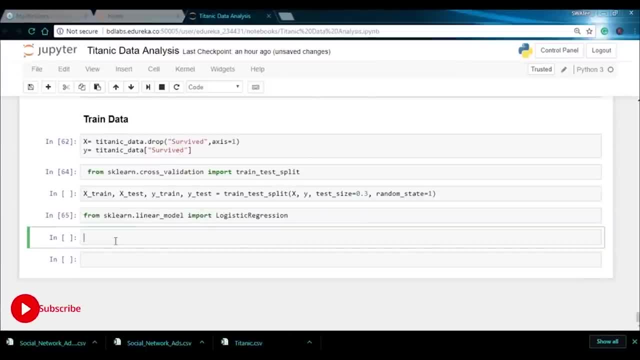 Import logistic regression. Next, I'll just create the instance of this logistic regression model. So I'll say log model is equals to logistic regression. Now I just need to fit my model. So I'll say log model dot fit and I'll just pass in my X train. 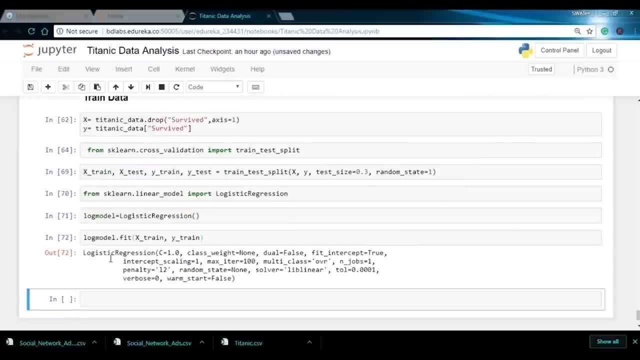 And Y train, All right. So here it gives me all the details of logistic regression. So here it gives me the class, weight, dual fit, intercept and all those things. then what I need to do? I need to make prediction, So I'll take a variable. 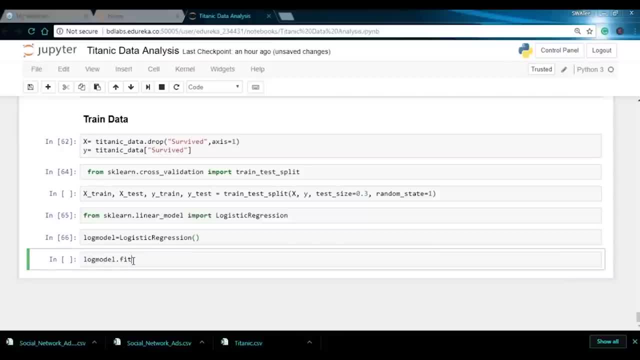 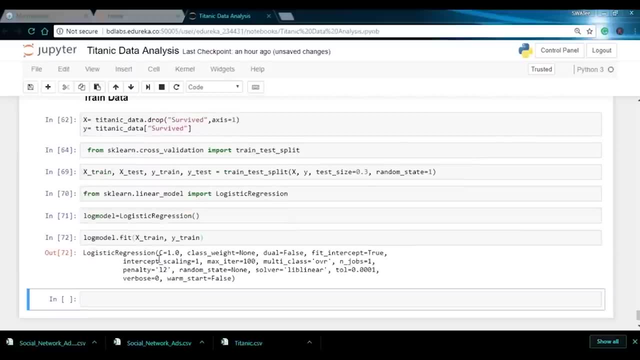 Now I just need to fit my model. So I'll say log model, dot fit, and I'll just pass in my x-train And y-train, All right. So here it gives me all the details of logistic regression. So here it gives me the class weight, dual fit, intercept and all those. 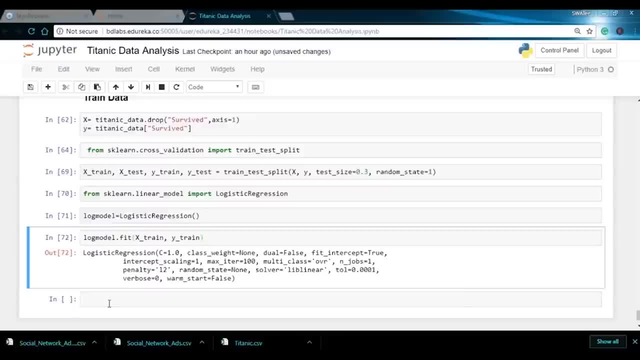 things. then what I need to do? I need to make prediction. So I'll take a variable, Let's say predictions, and I'll pass on the model to it. So I'll say log model, dot predict, and I'll pass in the value. 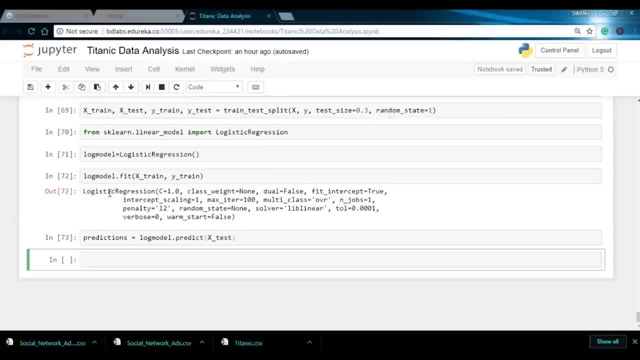 That is X test. So here we have just created a model. fit that model, and then we had made predictions. So now to evaluate how my model has been performing. so you can simply calculate the accuracy, or you can also calculate a classification report. So don't worry guys. 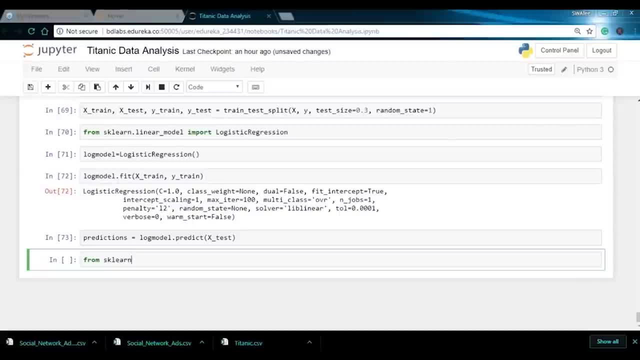 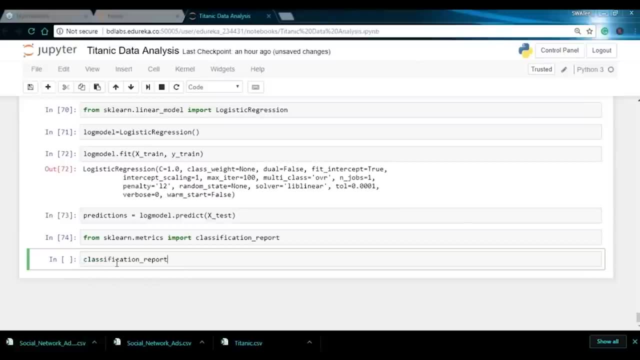 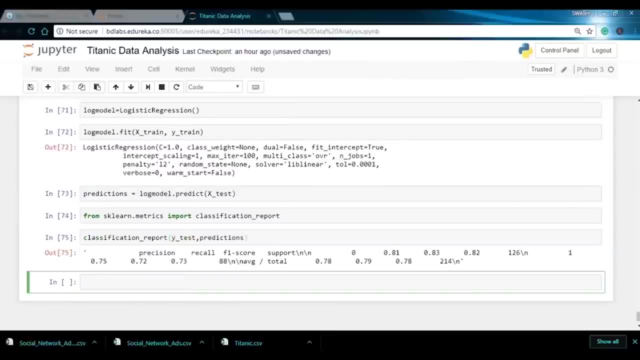 I'll be showing both of these methods. So I'll say from sklearn dot metrics Import classification report. So over here I use classification report And inside this I'll be passing in y test and the predictions. So, guys, this is my classification report. 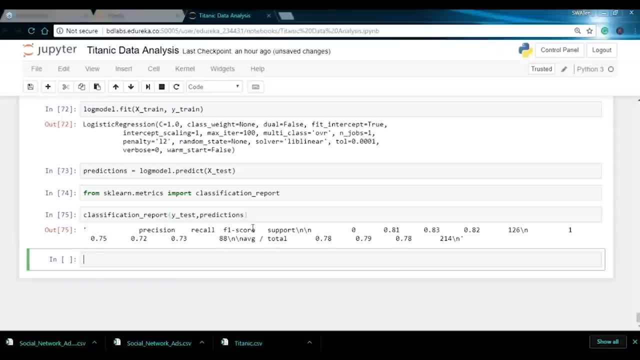 So over here I have the precision, I have the recall, We have the f1 score and then we have support. So here we have the value of precision as 75, 72 and 73, which is not that bad now, in order to calculate the accuracy as well. 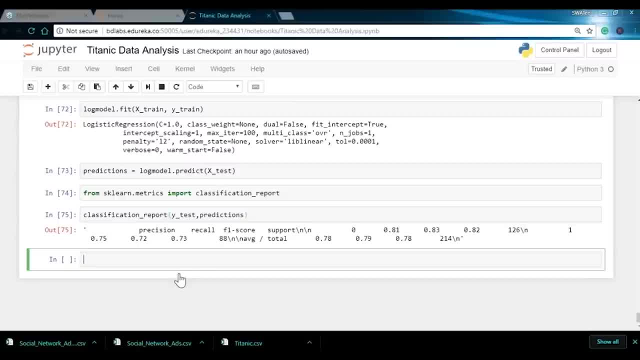 You can also use the concept of confusion matrix. So if you want to print the confusion matrix, I will simply say: from sklearn dot metrics, import confusion matrix first of all, and then we'll just print this. So here my function has been imported successfully. 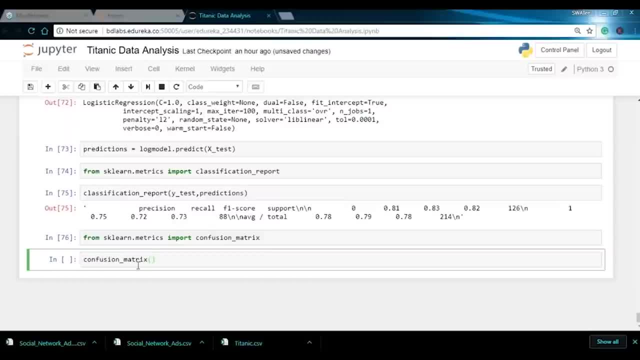 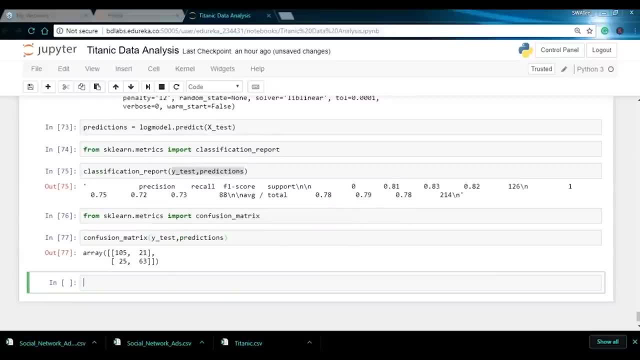 So I'll say confusion matrix And I'll again pass in the same variables, which is y test and predictions. So I hope you guys already know the concept of confusion matrix. So can you guys give me a quick confirmation as to whether you guys remember this confusion matrix concept or not? 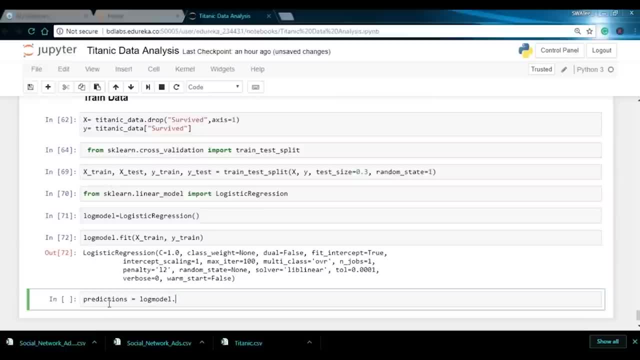 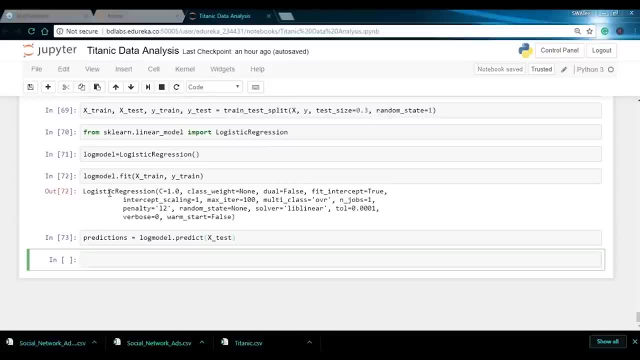 Let's say predictions and I'll pass on the model to it. So I'll say log model, dot predict, and I'll pass in the value That is X test. So here we have just created a model. fit that model, and then we had made predictions. 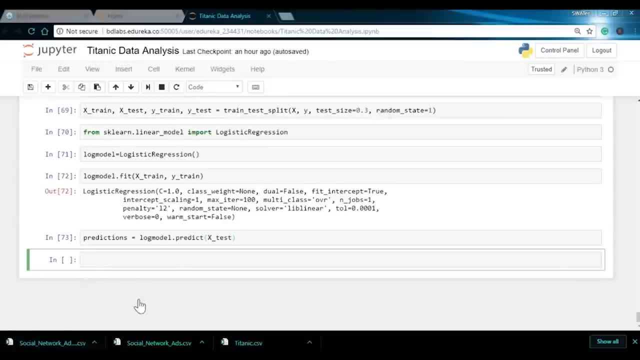 So now to evaluate how my model has been performing. so you can simply calculate the accuracy or you can also calculate a classification report. So don't worry guys, I'll be showing both of these methods. So I'll say: from sklearn dot metrics, Import classification report. 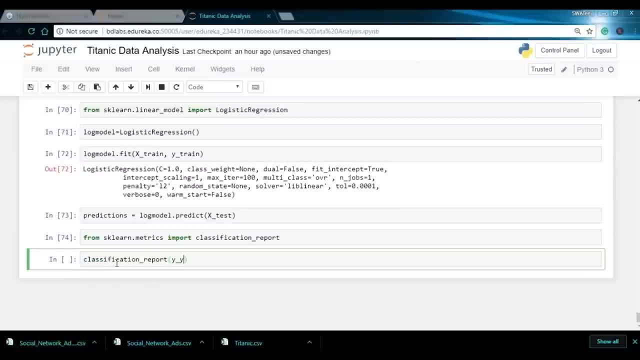 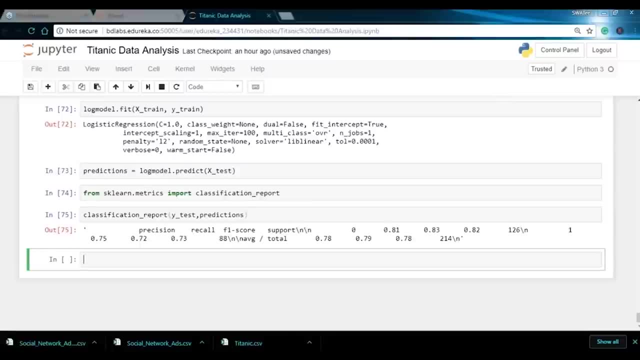 Over here I use classification report and inside this I'll be passing in y test and the predictions. So, guys, this is my classification report. So over here I have the precision, I have the recall, We have the F1 score and then we have support. 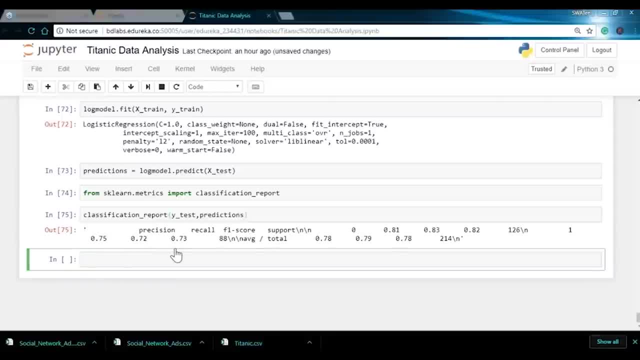 So here we have the value of precision as 75.. 72 and 73, which is not that bad. now, in order to calculate the accuracy as well, You can also use the concept of confusion matrix. So if you want to print the confusion matrix, I will simply. 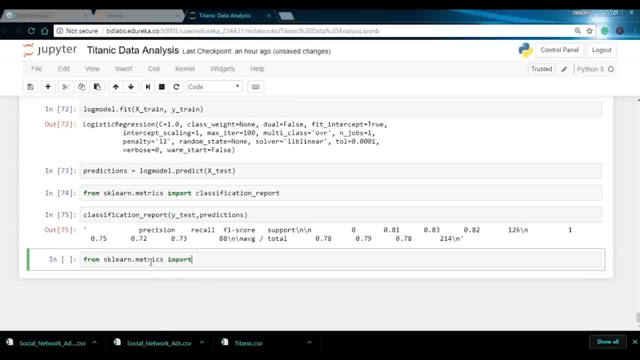 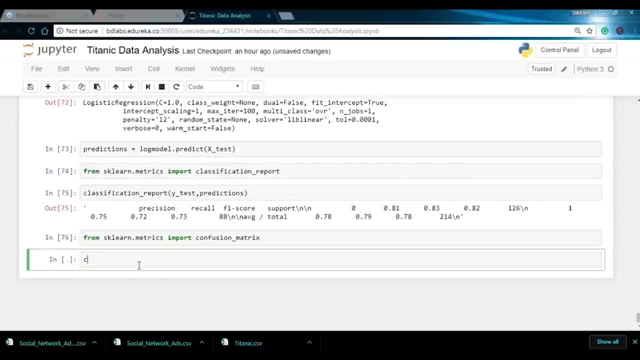 say from sklearn dot metrics, import, confusion matrix first of all, and then we'll just print this. So here my function has been imported successfully. So I'll say confusion matrix And I'll again pass in the same variables, which is y test and predictions. 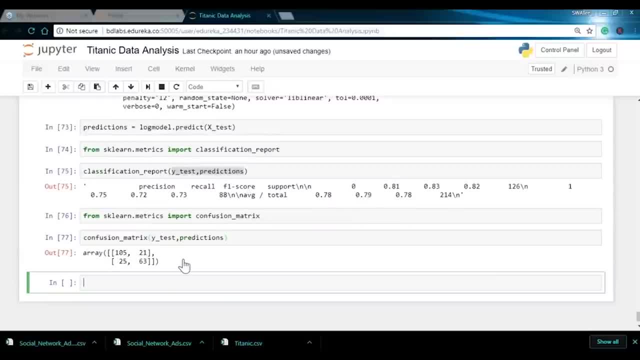 So I hope you guys already know the concept of confusion matrix. So can you guys give me a quick confirmation as to whether you guys remember this confusion matrix concept or not? So if not, I can just quickly summarize this as well. Okay, Jagruti says a yes. 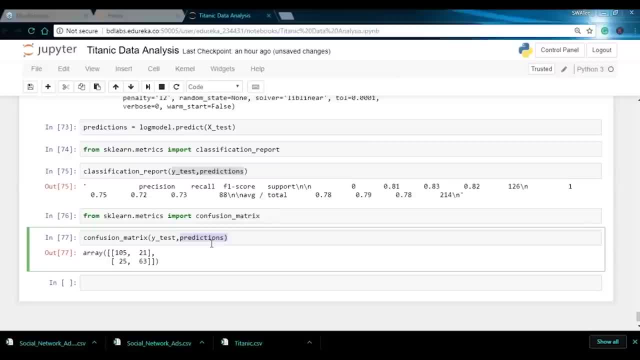 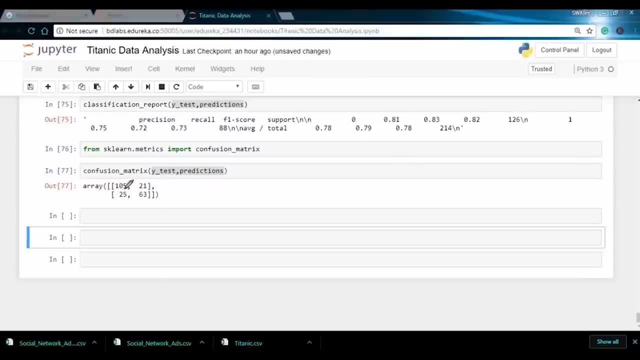 Okay, Swati is not clear with this, So I'll just tell you in a brief what confusion matrix is all about. So confusion matrix is nothing but a two by two matrix which has a four outcomes. This basically tells us that how accurate your values are. 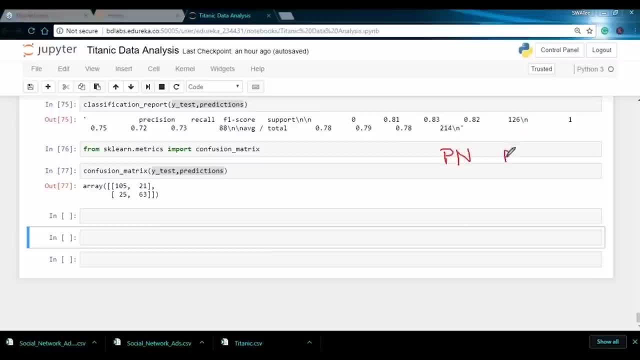 So here we have the column as predicted No, predicted y, And we have actual no and an actual yes. So this is the concept of confusion matrix. So here let me just feed in these values which we have just calculated. So here we have 105, 105, 21, 25 and 63. 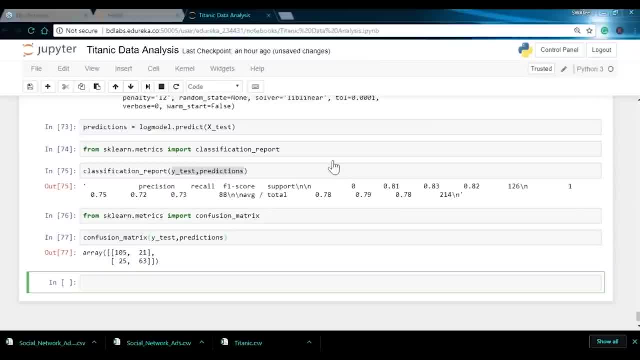 So, if not, I can just quickly summarize this as well. Okay, Jagruti says a yes. Okay, Swati is not clear with this. So I'll just tell you in a brief what confusion matrix is all about. So confusion matrix is nothing but a two by two matrix which has 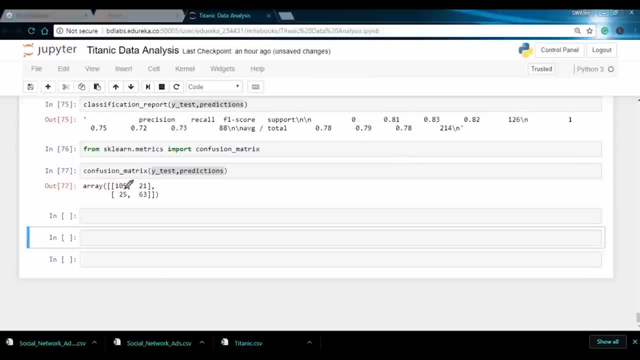 a four outcomes. This basically tells us that how accurate your values are. So here we have the column as predicted No, predicted y, and we have actual no and an actual yes. So this is the concept of confusion matrix. So here let me just feed in these values. 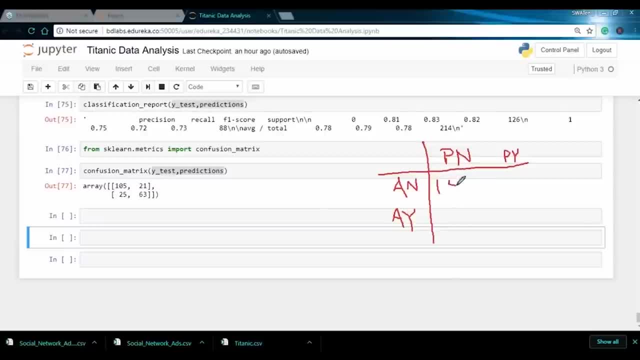 Which we have just calculated. So here we have 105, 105, 21, 25 and 63.. So, as you can see, here we have got four outcomes. Now, 105 is the value where a model has predicted no and in reality it was also a no. 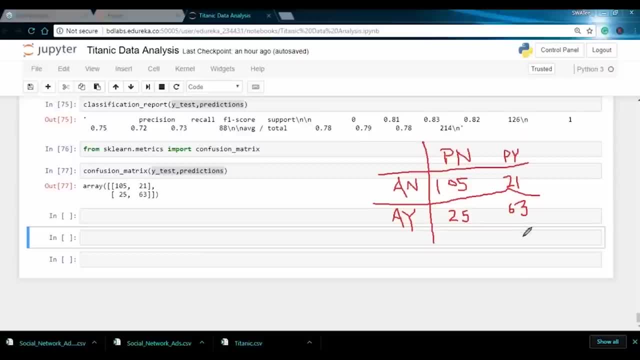 So here we have predicted no and an actual no. Similarly, we have 63 as a predicted Yes. So here the model predicted Yes and actually also it was a yes. So in order to calculate The accuracy, you just need to add the sum of these two values. 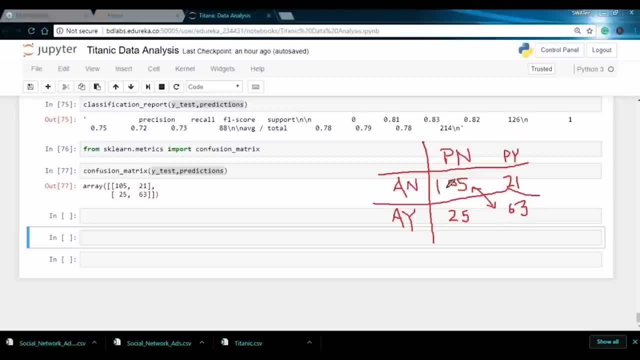 and divide the whole by the sum. So here these two values tells me where the model has actually predicted the correct output. So this value is also called as true negative. This is called as false positive. This is called as true positive and this is called as false negative. 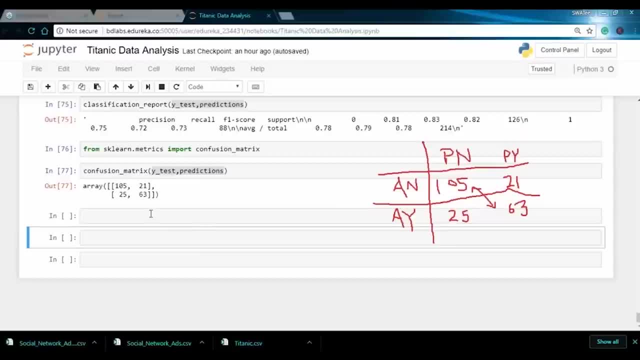 Now, in order to calculate the accuracy, don't have to do it manually. So in Python you can just import accuracy score function and you can get the results from that. So I'll just do that as well. So I'll say: from sklearncom. 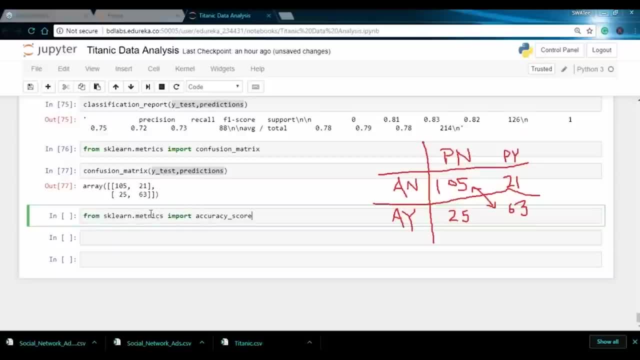 Dot metrics import accuracy score and I simply print the accuracy I will pass in the same variables, that is, y test and predictions. over here It tells me the accuracy as 78, which is quite good. So over here, if you want to do it manually, you have to plus these. 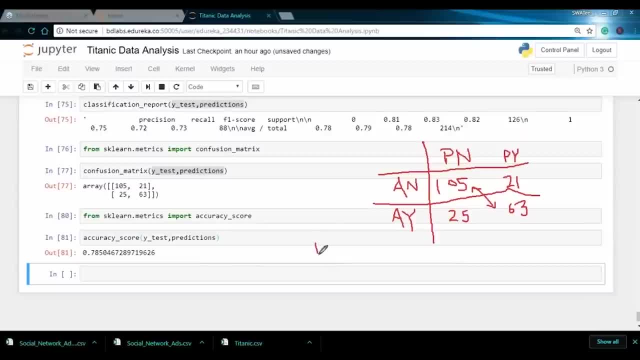 two numbers, which is 105 plus 63.. So this comes out to almost 168, and then you have to divide it by the sum of all the four numbers, So 105 plus 63 plus 21 plus 25.. So this gives me a result of 214.. 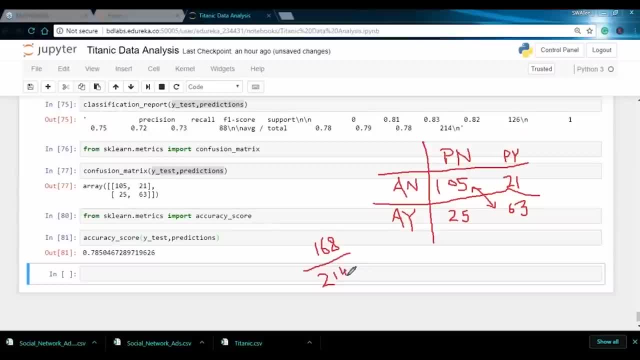 So now, if you divide these two number, you'll get the same accuracy, that is, 78%, or you can say 0.78.. So that is how you can calculate the accuracy. So now let me just go back to my presentation and let's see what. 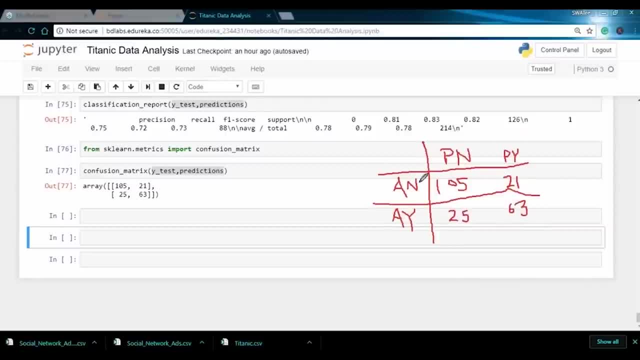 So, as you can see here, we have got four outcomes. Now, 105 is the value where our model has predicted No and in reality it was also a no, So where we have predicted no and an actual no. Similarly, we have 63 as a predicted 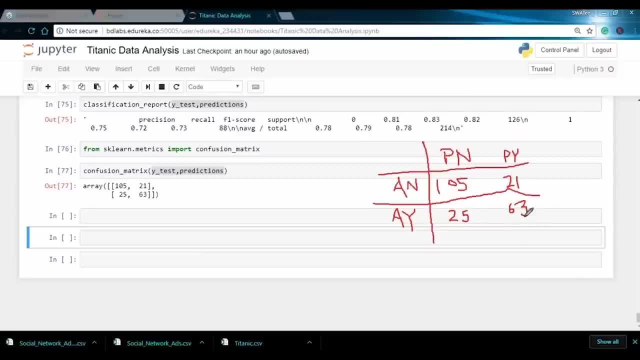 Yes. So here the model predicted Yes, and actually also it was a yes. So in order to calculate the accuracy, you just need to add the sum of these two values and divide the whole by the sum. So here these two values tells me where the model has actually predicted. 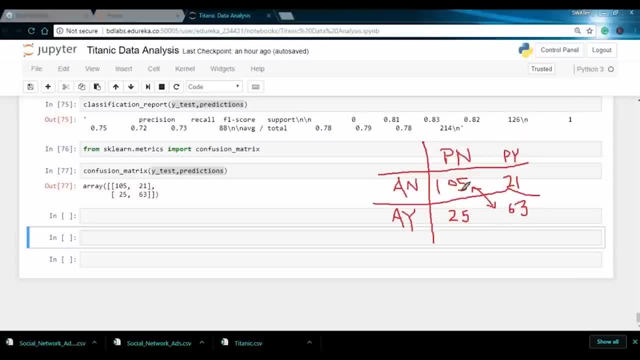 the correct output. So this value is also called as true negative, This is called as false positive, This is called as true positive And this is called As false negative. now, in order to calculate the accuracy, don't have to do it manually. 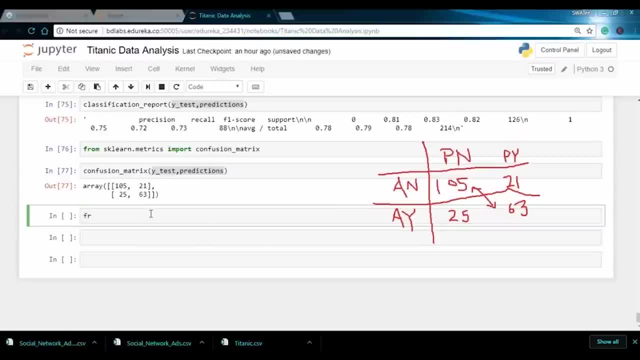 So in Python you can just import accuracy score function and you can get the results from that. So I'll just do that as well. So I'll say: from sklearnmetrics import accuracy score and I simply print the accuracy. I will pass in the same variables. that is why test and predictions. 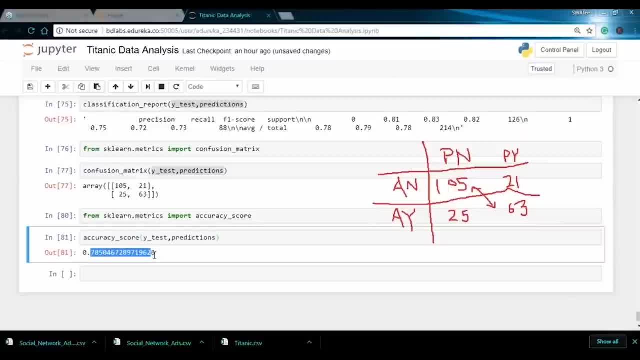 over here It tells me the accuracy as 78, which is quite good. So over here, if you want to do it manually, You have to plus these two numbers, which is 105 plus 63. So this comes out to almost 168, and then you have to divide by the sum. 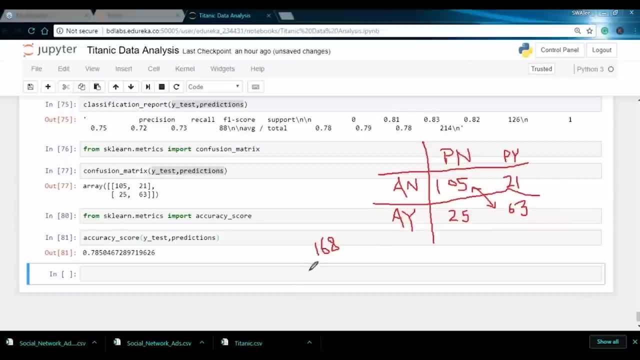 of all the four numbers, So 105 plus 63 plus 21 plus 25.. So this gives me a result of 214.. So now, if you divide these two number, you'll get the same accuracy, that is 78%, or you can say 0.78.. 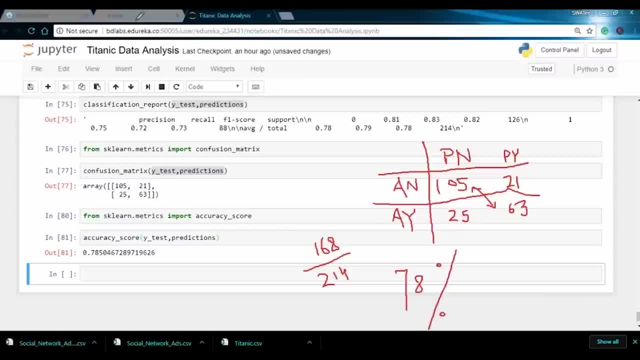 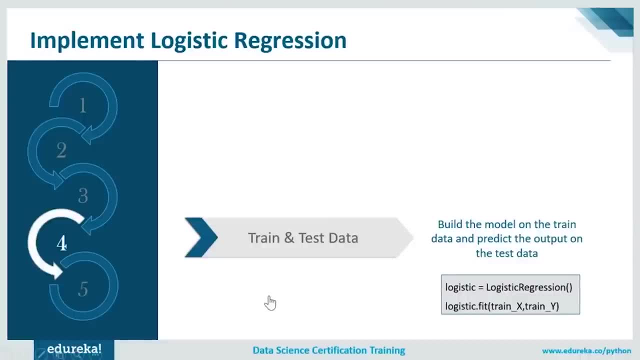 So that is how you can calculate the accuracy. So now let me just go back to my presentation and let's see what all we have covered till now. So here we have first split our data into train and test subset. Then we have build our model on the train data and then predicted. 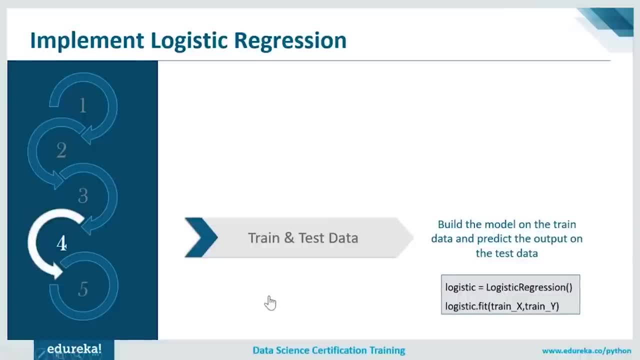 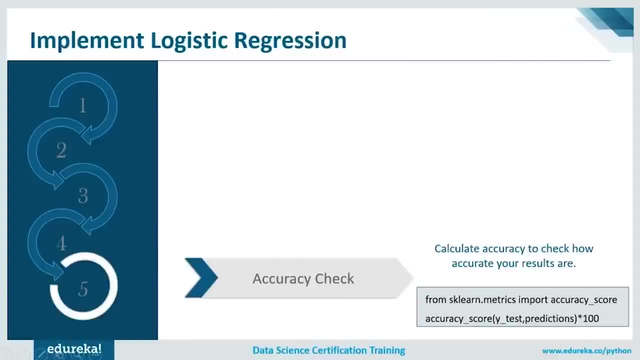 all we have covered till now. So here we have first split our data into train and test subset, Then we have build our model on the train data and then predicted the output on the test data set. and then my fifth step is to check the accuracy. 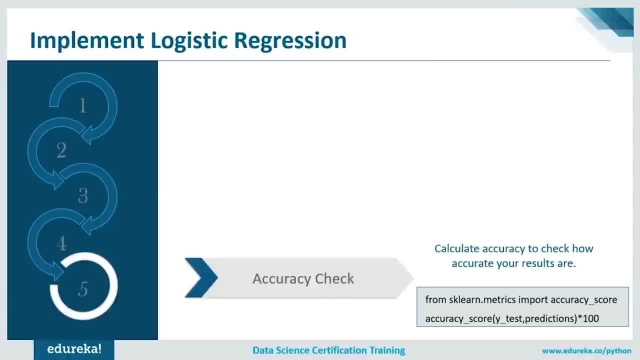 So here we have calculated accuracy to almost 78. percent, which is quite good. You cannot say that accuracy is bad. So here it tells me how accurate your results are. So here my accuracy score defines that, and hence we got a good accuracy. 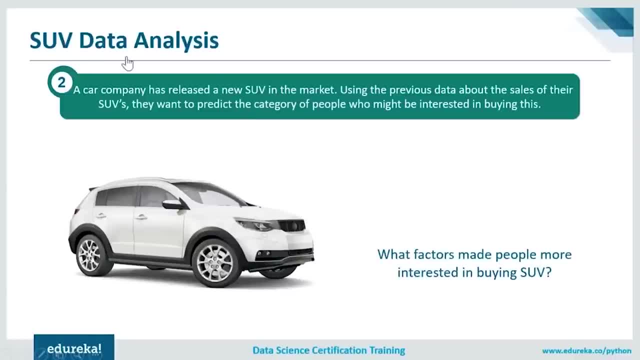 So now moving ahead, let us see the second project, that is, SUV data analysis. So in this, a car company has released new SUV in the market and, using the previous data about the sales of their SUV, They want to predict the category of people who might be. 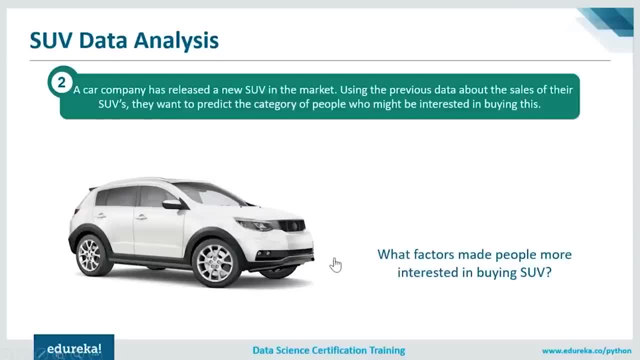 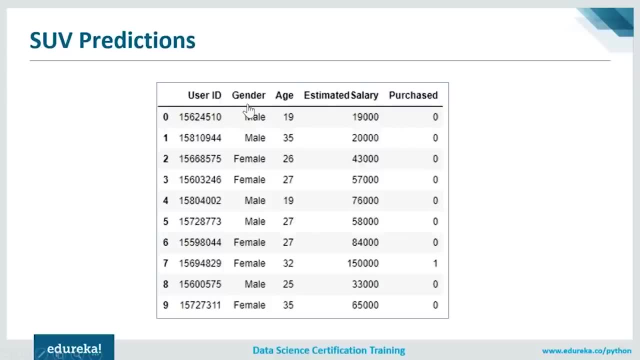 interested in buying this. So, using the logistic regression, you need to find what factors made people more interested in buying this SUV. So for this, let us see a data set where I have user ID, I have gender as male and female, then we have the age we have. 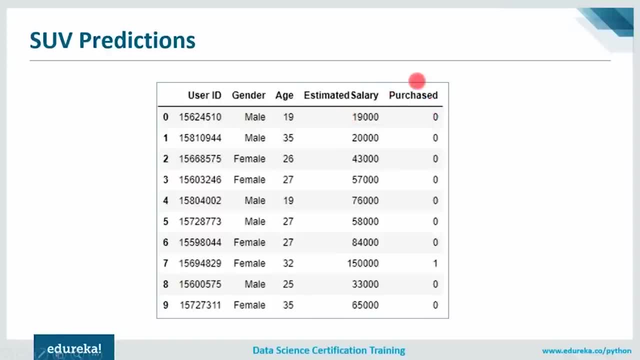 the estimated salary, and then we have the purchase column. So this is my discrete column, or you can say the categorical column. So here we just have the value, that is, 0 and 1, and this column. we need to predict whether a person can actually purchase a. 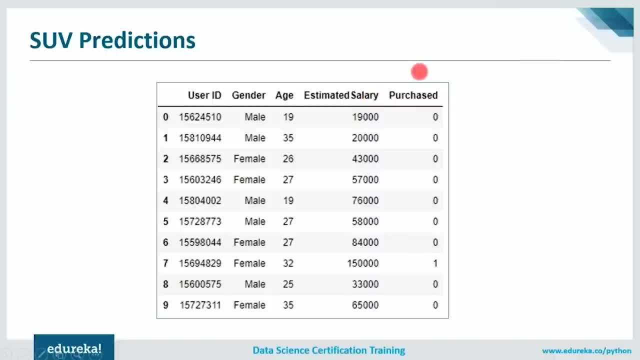 SUV or not. So based on these factors, we will be deciding whether a person can actually purchase a SUV or not. So we know the salary of a person, We know the age and using these we can predict whether person can actually purchase SUV or not. 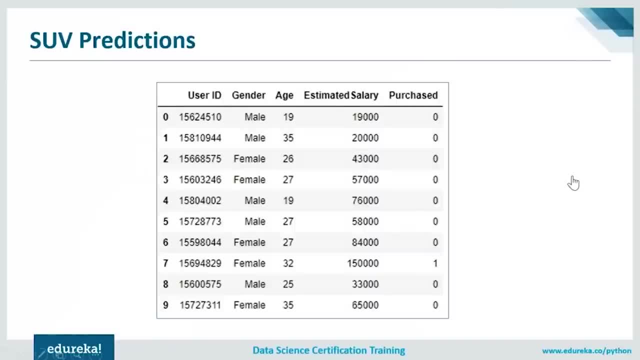 So let me just go to my Jupyter notebook and let us implement logistic regression. So, guys, I will not be going through all the details of data cleaning and analyzing the part. that part, I'll just leave it on you. So just go ahead and practice as much as you can. 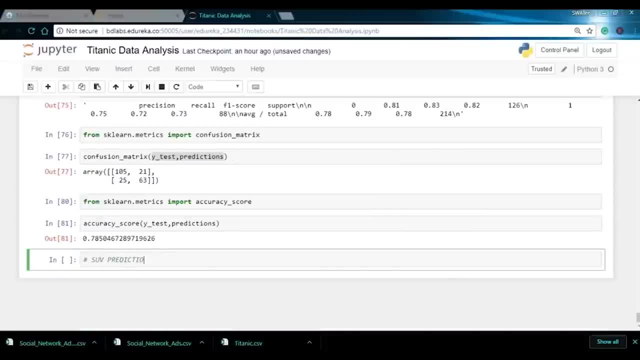 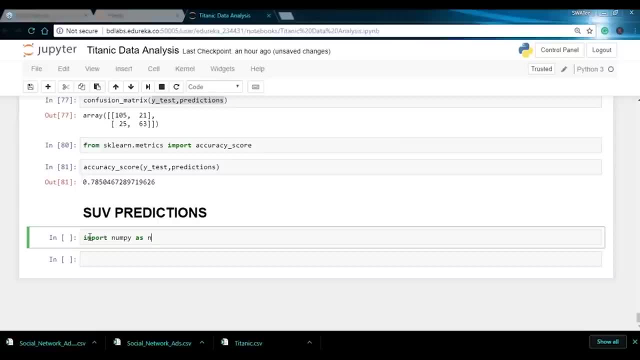 All right. So my second project is SUV predictions. All right, So first of all I have to import all the libraries. So I say import numpy as n, P and similarly I'll do the rest of it. All right, So now let me just print the head of this data set. 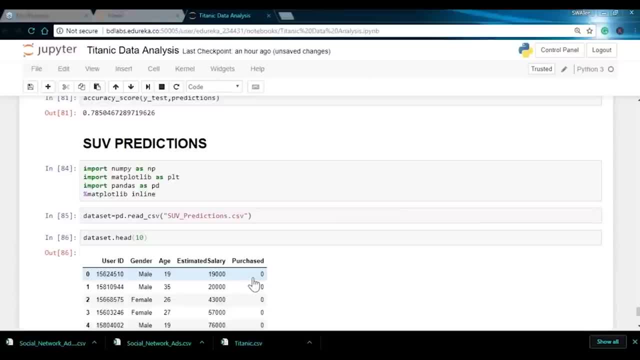 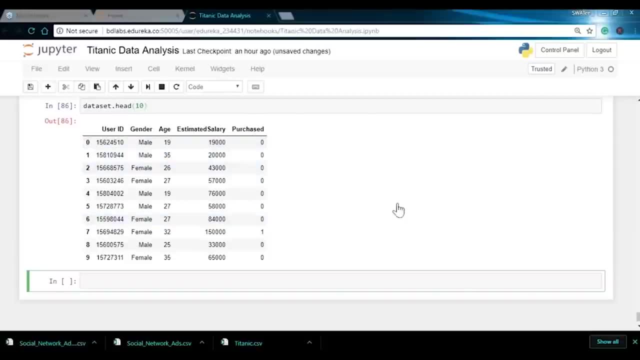 So this we've already seen that we have columns as user ID, We have gender, we have the age, we have the salary and then we have to calculate whether person can actually purchase a SUV or not. So now it is just simply go on to the algorithm part. 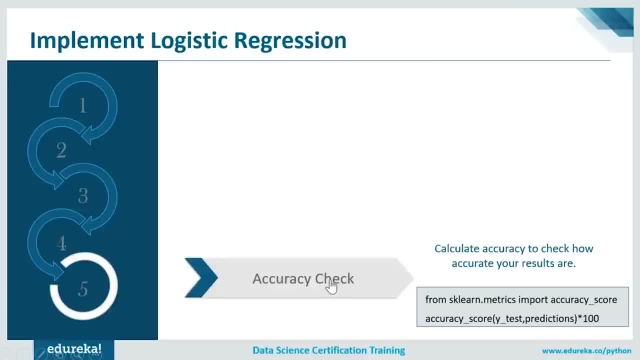 the output on the test data set. and then my fifth step is to check the accuracy. So here we have calculated accuracy to almost 78%, which is quite good. You cannot say that accuracy is bad. So here it tells me how accurate your results are. 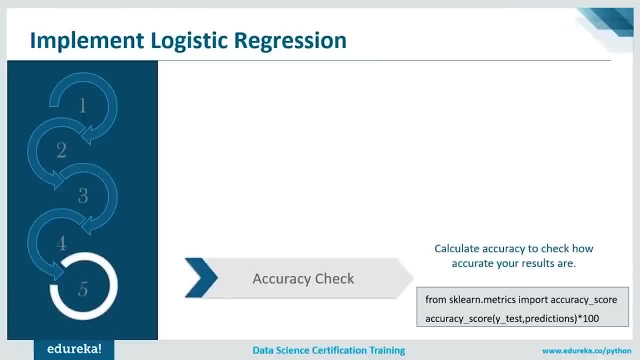 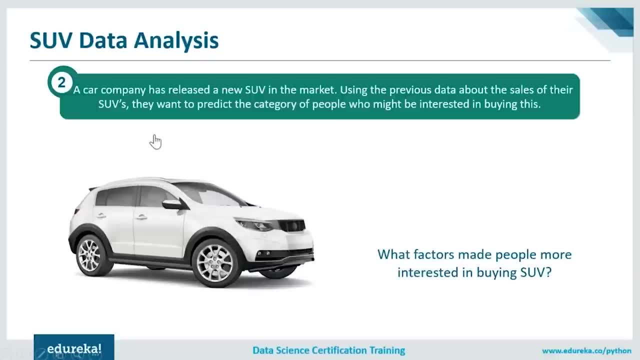 So here my accuracy score defines that, and hence we got a good accuracy. So now moving ahead. Let us see the second project, that is, SUV data analysis. So in this, a car company has released new SUV in the market and using the previous data about the sales of their SUV, 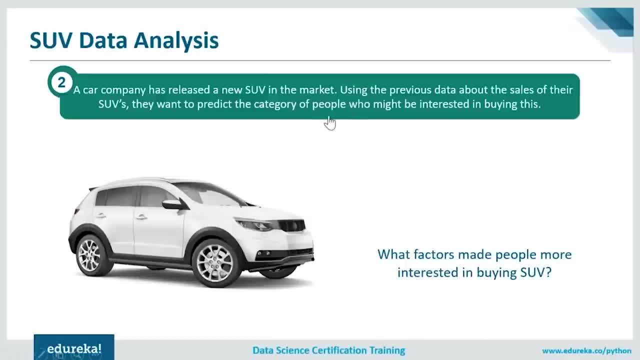 They want to predict the category of people who might be interested in buying this. So, using the logistic regression, you need to find what factors made people more interested in buying this SUV. So for this, let us see a data set where I have user ID. 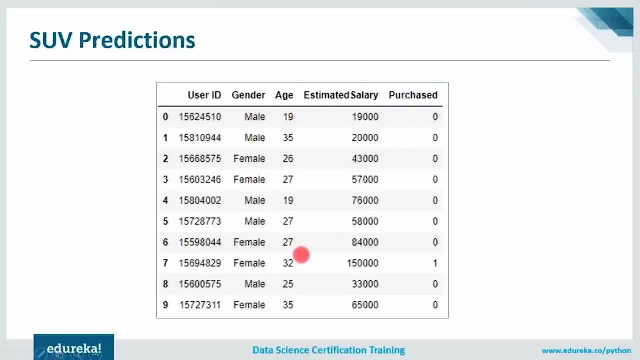 I have gender as male and female, then we have the age, we have the estimated salary and then we have the purchase column. So this is my discrete column. I can see the categorical column. So here we just have the value, that is, 0 and 1, and this column. 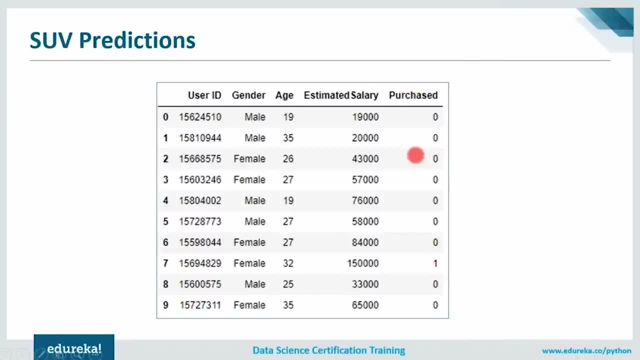 we need to predict whether a person can actually purchase a SUV or not. So, based on these factors, we will be deciding whether a person can actually purchase a SUV or not. So we know the salary of a person, We know the age and using these, we can predict whether person 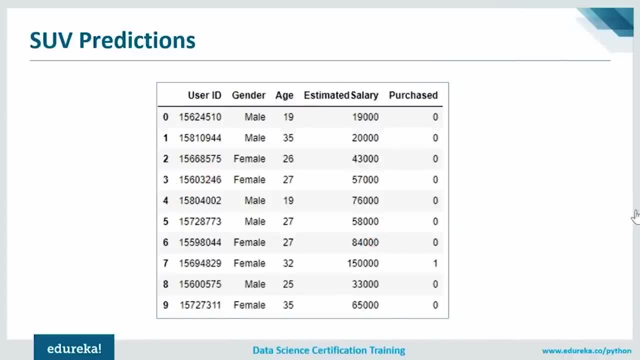 can actually purchase SUV or not. So let me just go to my Jupiter notebook and implement logistic regression. So, guys, I will not be going through all the details of data cleaning and analyzing the part. that part I'll just leave it on you. So just go ahead and practice as much as you can. 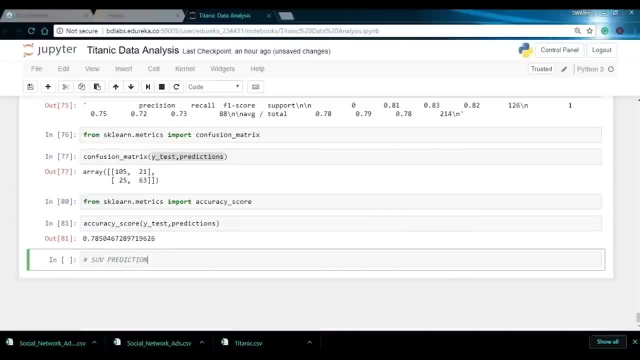 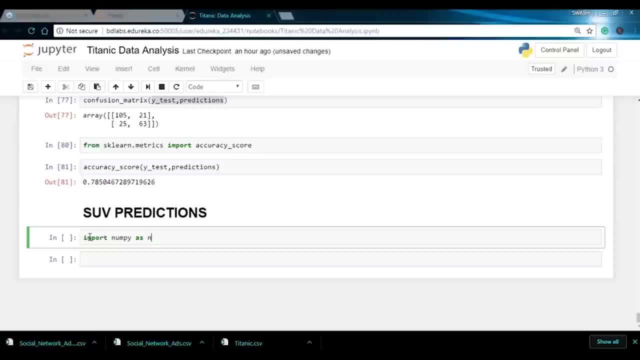 All right. So my second project is SUV predictions. All right. So first of all I have to import all the libraries, So I say import numpy as NP and similarly I'll do the rest of it. All right. So now let me just print the head of this data set. 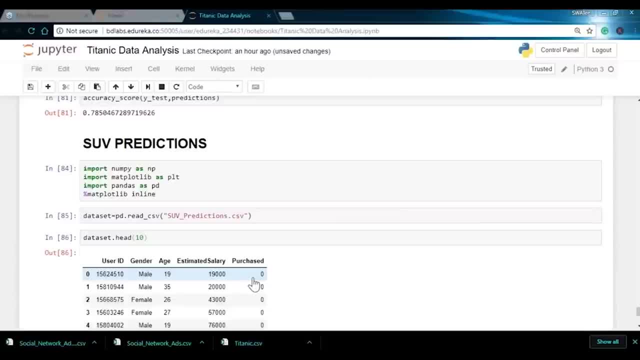 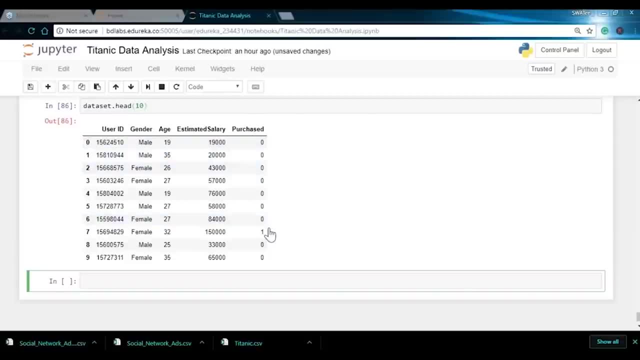 So this we've already seen that We have columns as user ID, We have gender, We have the age, We have the salary and then we have to calculate whether person can actually purchase a SUV or not. So now it is just simply go on to the algorithm part. 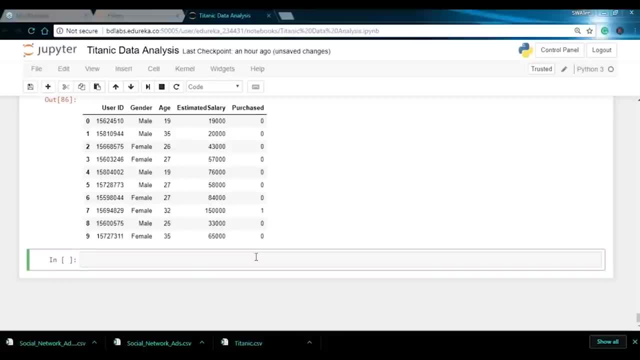 So we'll directly start off with the logistic regression or how you can train a model. So for doing all those things, we first need to define your independent variable and dependent variable. So in this case, I want my x. that is an independent variable. 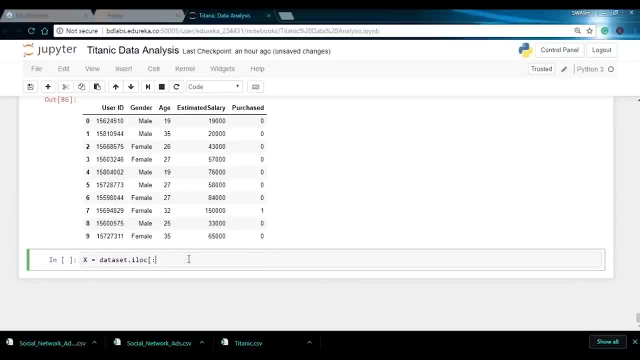 I said data set, dot I lock. So here I'll be specifying all the rows. So colon basically stands for That and in the columns I want only two and three dot values. So here should fetch me all the rows and only the second and 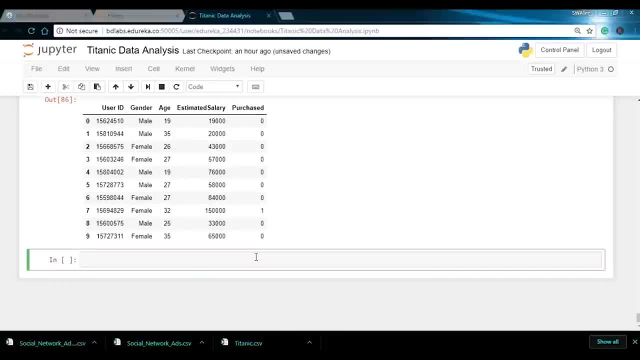 So we'll directly start off with the logistic regression, How you can train a model. So for doing all those things, we first need to define your independent variable and dependent variable. So in this case, I want my x. that is an independent variable. 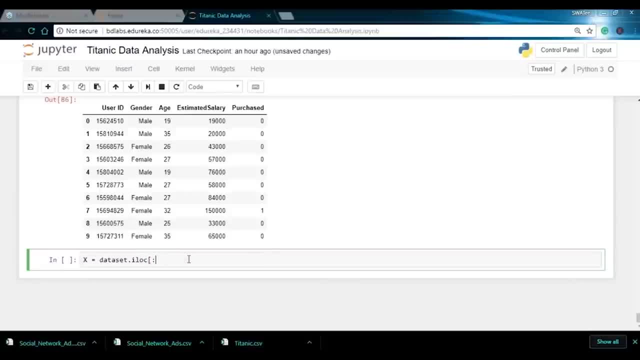 I said data set, dot I lock. So here I'll be specifying all the rows. So colon basically stands for that and in the columns I want only two and three dot values. So here should fetch me all the rows and only the second and 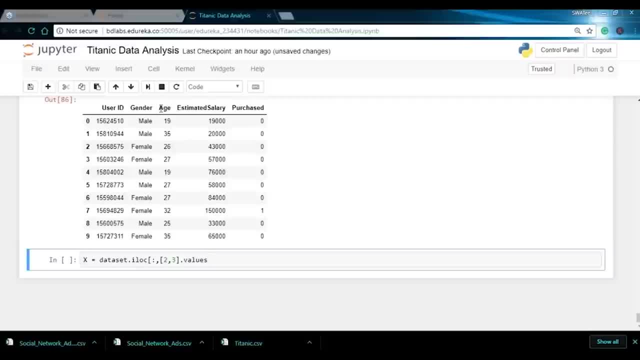 third column, which is age and estimated salary. So these are the factors which will be used to predict the dependent variable that is purchase. So here my dependent variable is purchase and independent variable is of age and salary. So I'll say data set dot. 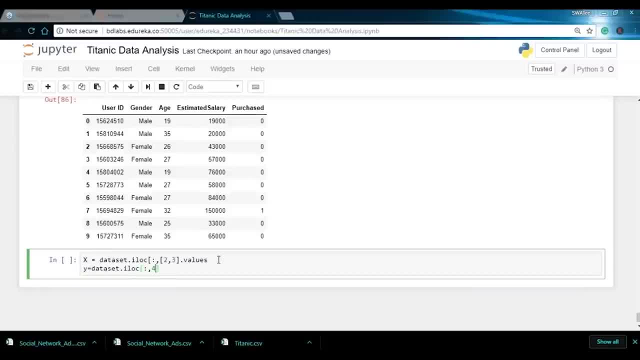 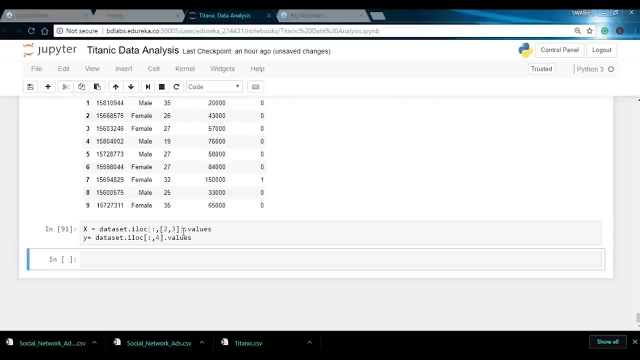 I love, I'll have all the rows and I just want fourth column, That is, my purchased column- dot values, All right, So I've just forgot one one square bracket over here, All right. So over here I have defined my independent variable and dependent. 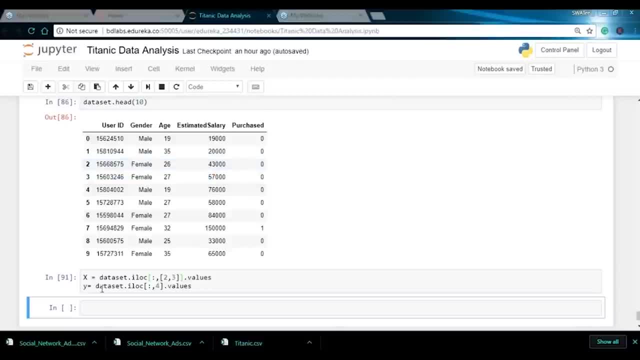 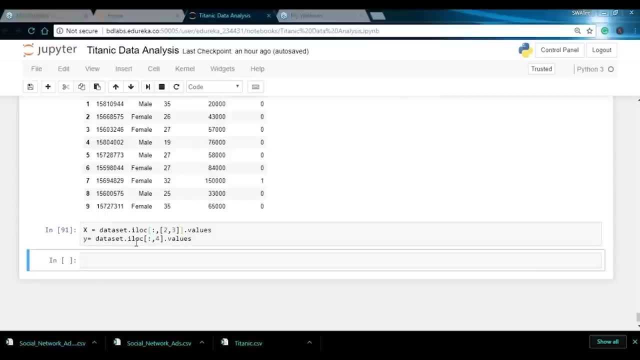 variable. So here my independent variable is age and salary and dependent variable is the column purchase. Now you must be wondering: what is this? I log function, So I love. function is basically an indexer for Pandas data frame and it is used for integer based indexing. 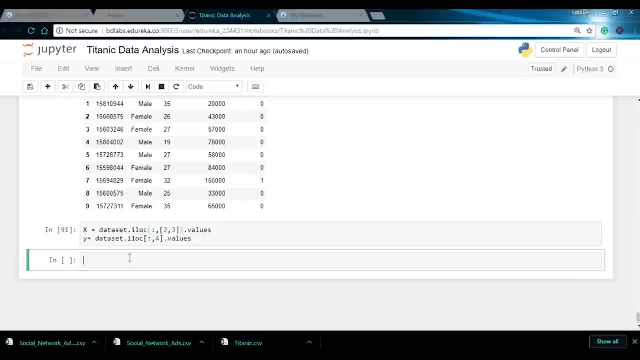 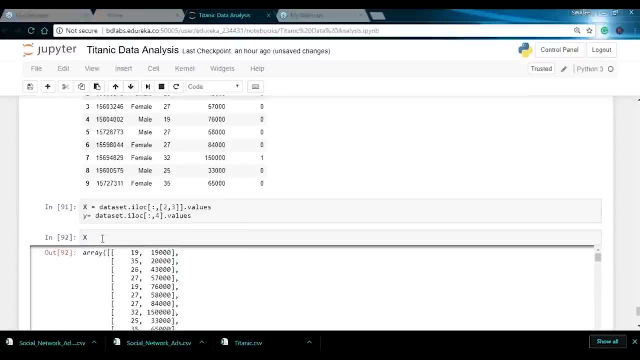 I can also say selection by index. Now let me just print these independent variables and dependent variable. So if I print the independent variable, I have the age as well as the salary. next Let me print the dependent variable as well. So over here you can see I just have the values in 0 and 1, so 0. 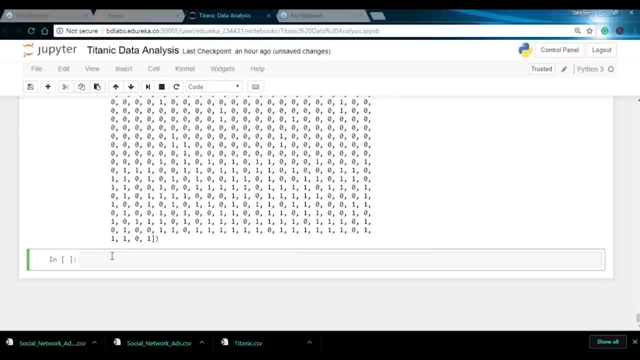 stands for did not purchase. next, Let me just divide my data set into training Test subset, So I'll simply write in from sklearn dot cross, split dot cross- validation- Import train test. Next, I just press shift and tab and over here. 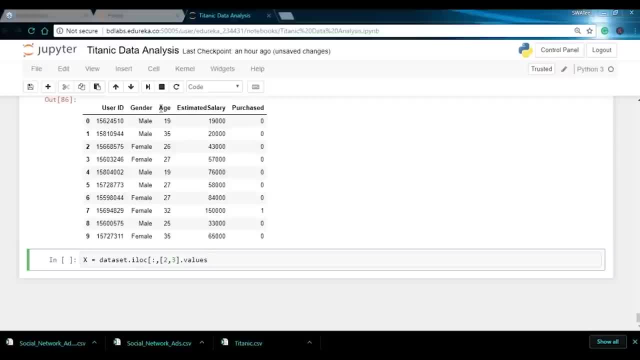 third column, which is age and estimated salary. So these are the factors which will be used to predict the dependent variable that is purchase. So here my dependent variable is purchase and independent variable is of age and salary. So I'll say data set dot. 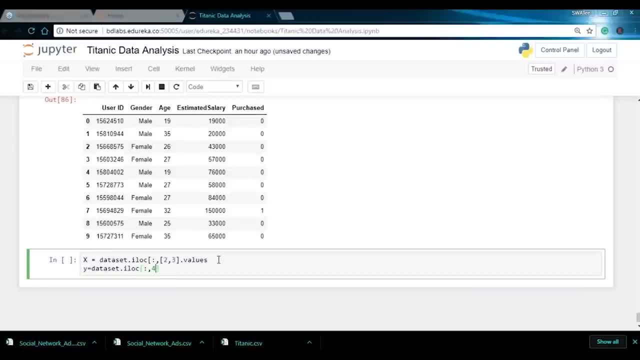 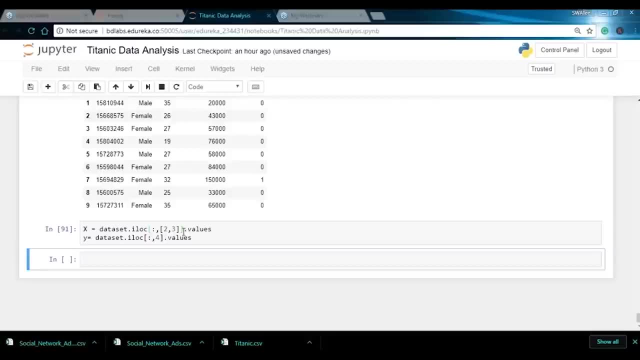 I love, I'll have all the rows and I just want fourth column, That is, my purchased column- dot values, All right, So I've just forgot one one square bracket over here, All right. So over here I have defined my independent variable and dependent. 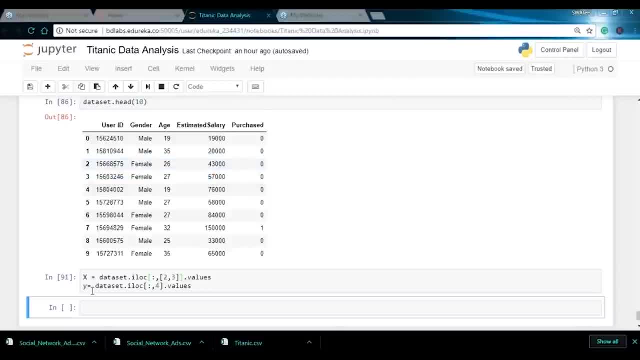 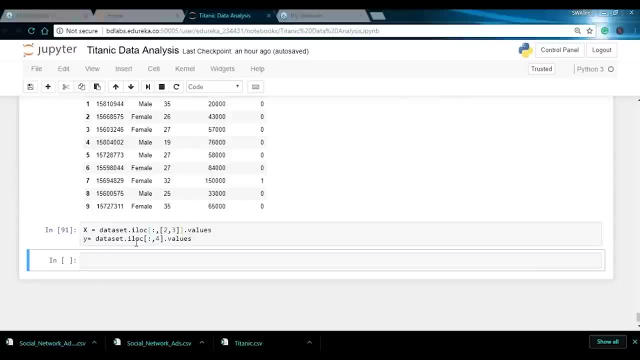 variable. So here my independent variable is age and salary and dependent variable is the column purchase. Now you must be wondering: what is this? I log function, So I love. function is basically an indexer for Pandas data frame and it is used for integer based indexing. 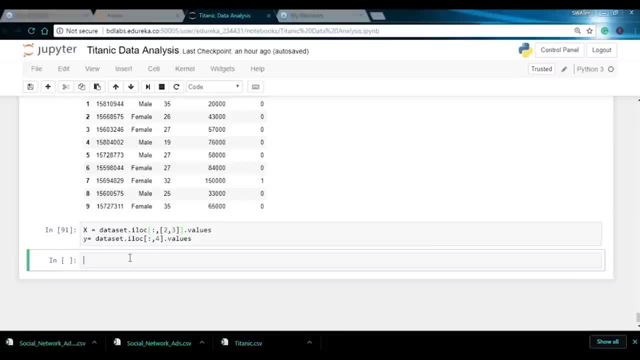 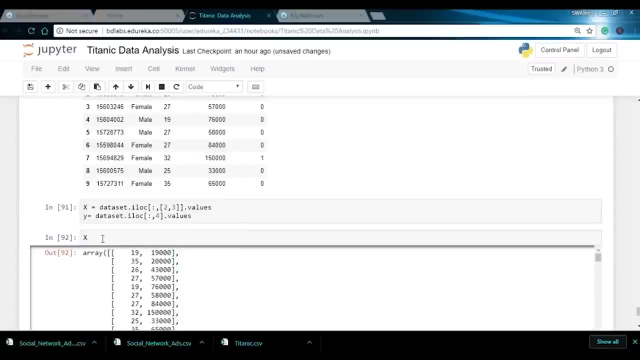 I can also say selection by index. Now let me just print these independent variables and dependent variable. So if I print the independent Variable I have the age as well as the salary. next Let me print the dependent variable as well. So over here you can see I just have the values in 0 and 1.. 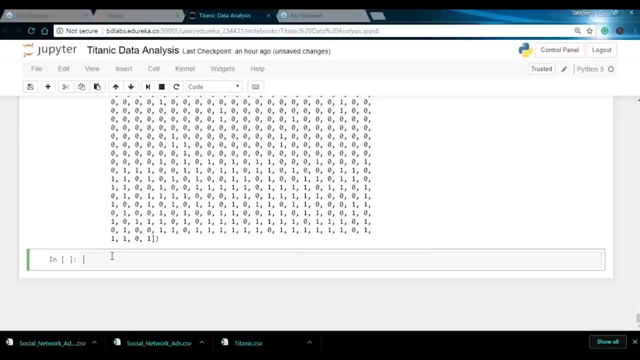 So 0 stands for did not purchase. next, Let me just divide my data set into training and test subset, So I'll simply write in from sklearn: dot cross, split dot cross, validation Import train test. Next, I just press shift and tab and over here. 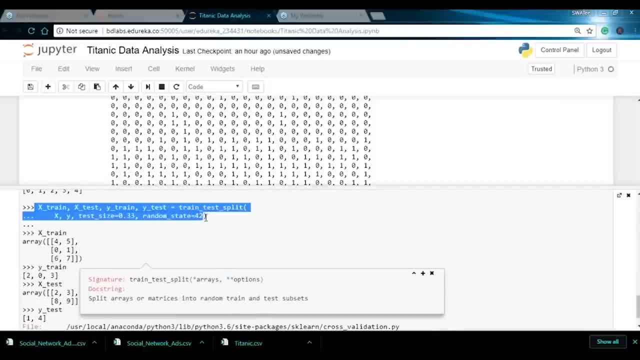 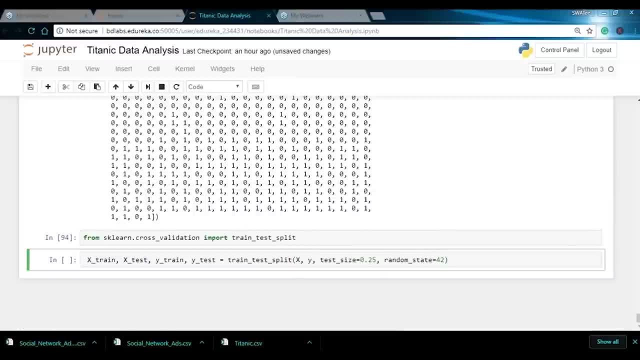 I'll go to the examples and just copy the same line. So I'll just copy this. I'll remove the points. Now I want the text size to be, let's say, 25.. So I have divided the train and test it in 7525 ratio. 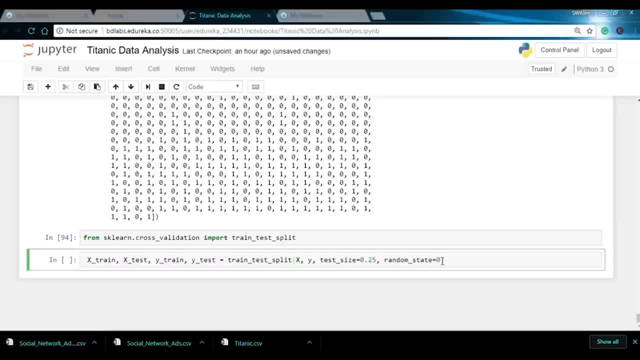 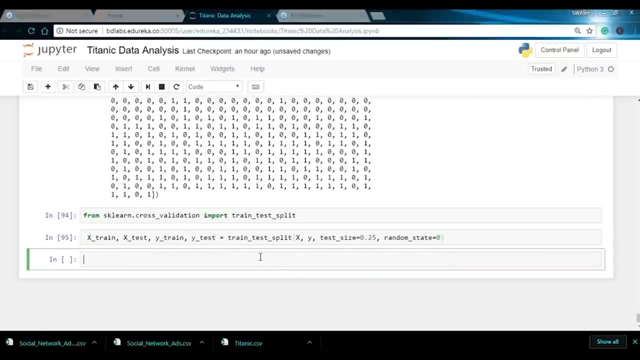 Now let's say I'll take the random set as 0, so random state basically ensures the same result, or you can say the same samples taken whenever you run the code. So let me just run this now. You can also scale your input values for better performing and. 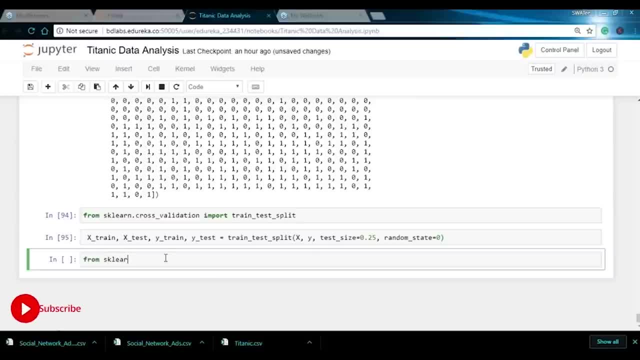 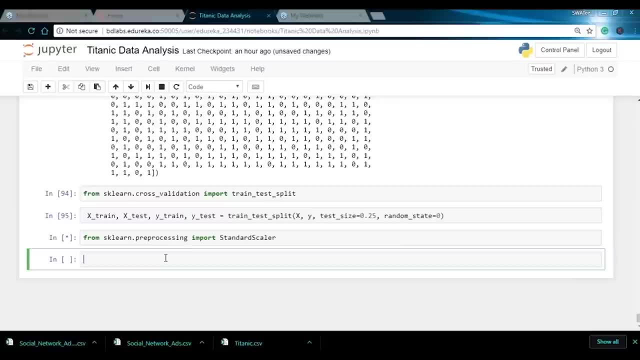 this can be done using standard scalar, So let me do that as well. So I'll say: from sklearn Dot pre-processing, Import standard scalar. Now why do we scale it? now? If you see a data set, we are dealing with large numbers. 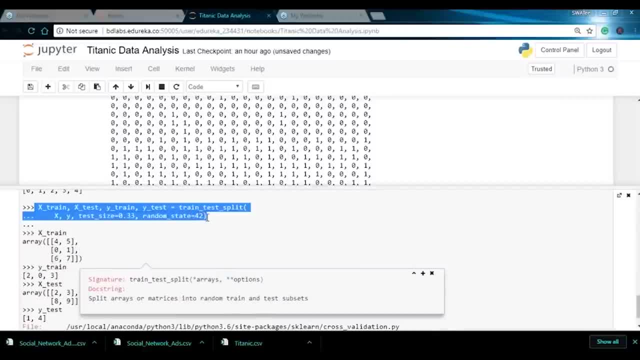 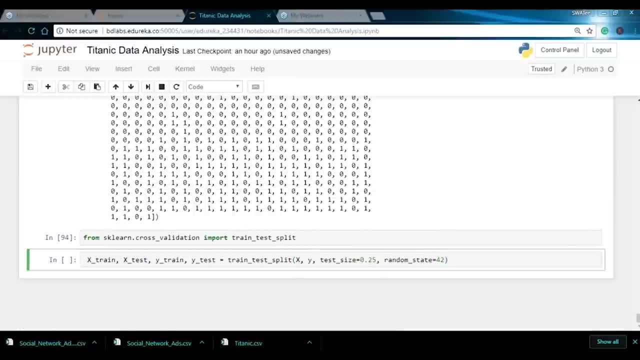 I'll go to the examples and just copy the same line. So I'll just copy this. I'll remove the points. now I want the text size to be, let's say, 25.. So I have divided the train and tested in 7525 ratio. 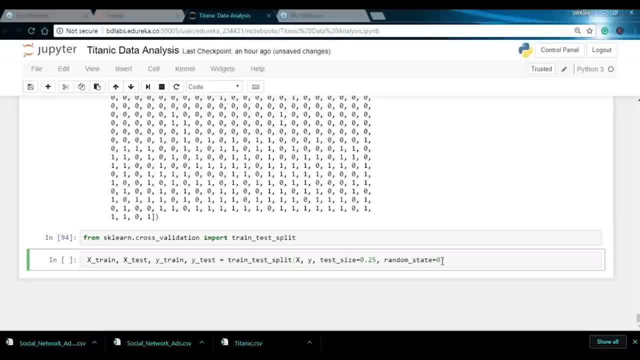 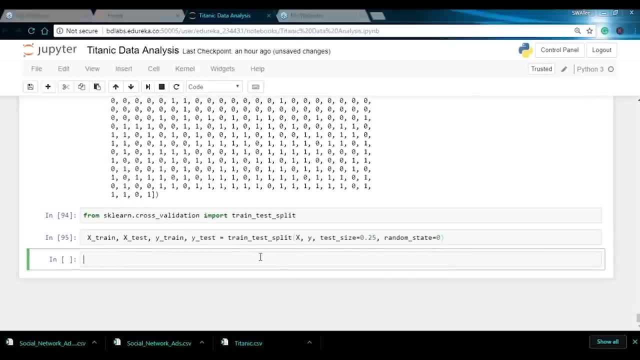 Now let's say I'll take the random set as 0. So random state basically ensures the same result. or you can say same samples taken whenever you run the code. So let me just run this now. You can also scale your input values for better performing. 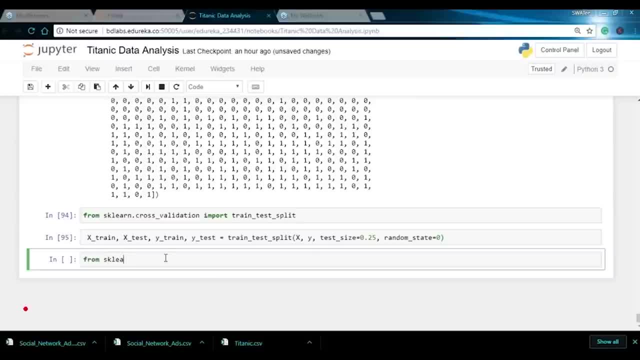 and this can be done using standard scalar. So let me do that as well. So I'll say: from sklearn dot pre-processing, Import standard scalar. Now why do we scale it? now, If you see a data set, we are dealing with large numbers. 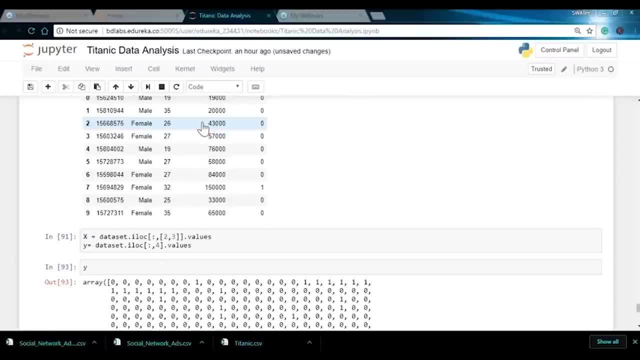 Well, although we are using a very small data set. So whenever you're working in a broad environment, you'll be working with large data set where you'll be using thousands and hundred thousands of duples, So they're scaling down will definitely affect the performance. 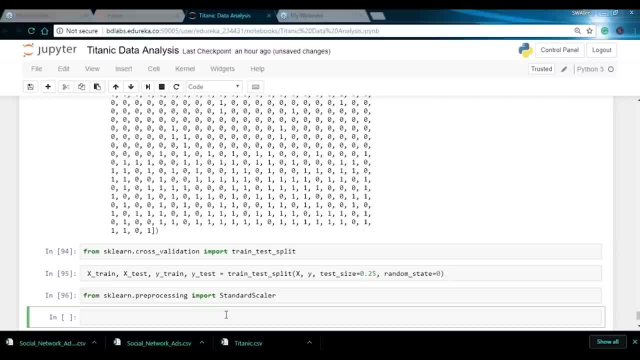 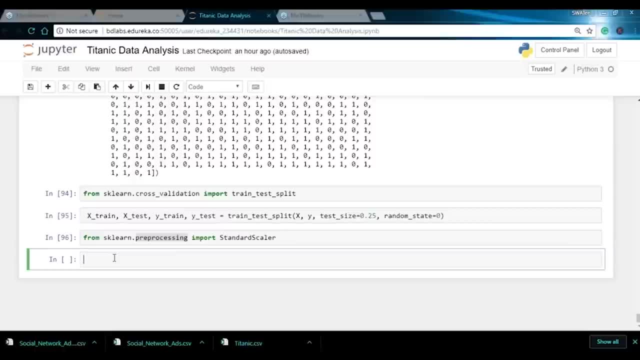 by a large extent. So here let me just show you how we can scale down these input values. and then the pre-processing contains all your methods and functionality which is required to transform your data. So now that is scaled down for test as well as a training data. 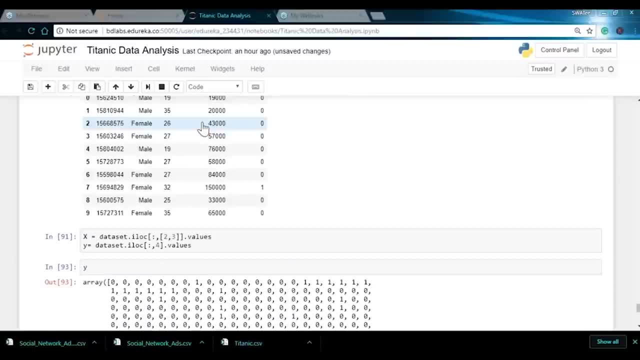 Well, although we are using a very small data set. So whenever you're working in a prod environment, you'll be working with large data set where you'll be using thousands and hundred thousands of tuples, So they're scaling down will definitely affect the performance. 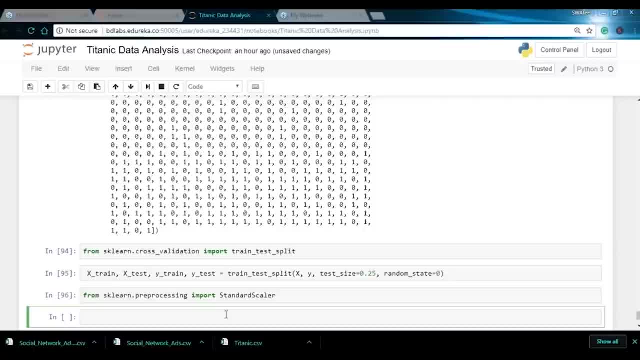 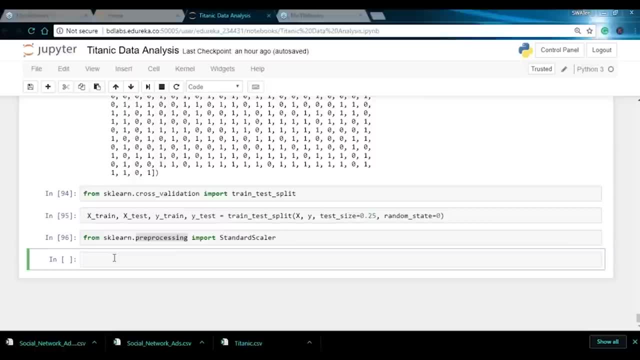 by a large extent. So here let me just show you how you can scale down these input values, and then the pre-processing contains all your methods and functionality which is required to transform your data. So now it is scaled down for test as well as a training data. 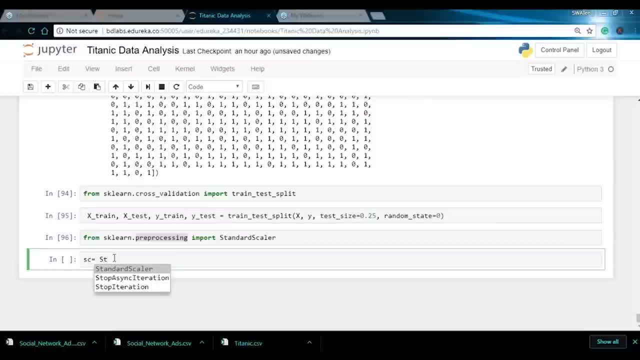 set. So I'll first make an instance of it. So I'll say standard scalar, then I'll have extreme. I'll say SC, dot, fit, fit, underscore, transform, I'll pass in my extreme variable. And similarly I can do it for test, where in I'll pass the X test. 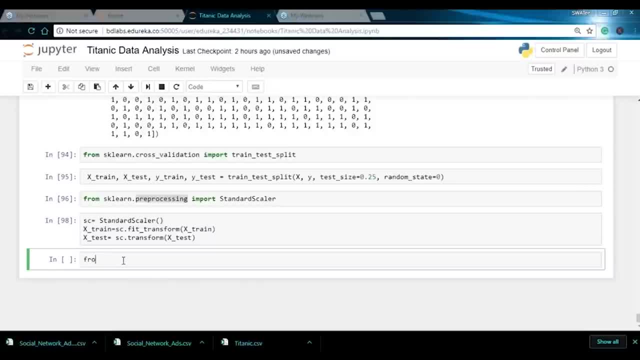 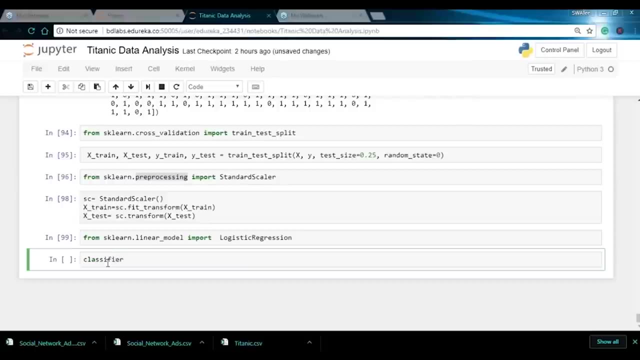 Now my next step is to import logistic regression. So I'll simply apply logistic regression by first importing it. So I'll say: from sklearn, from sklearn dot, linear model, import logistic regression. Over here I'll be using classifier, So I'll say: classifier dot is equals to logistic regression. 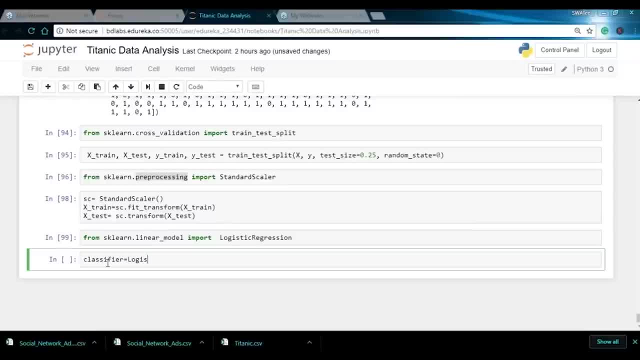 So over here I'll just make an instance of it. So I'll say logistic regression and over here I just pass in the random state which is zero, And now I'll simply fit the model And I simply pass in extreme and y-train. 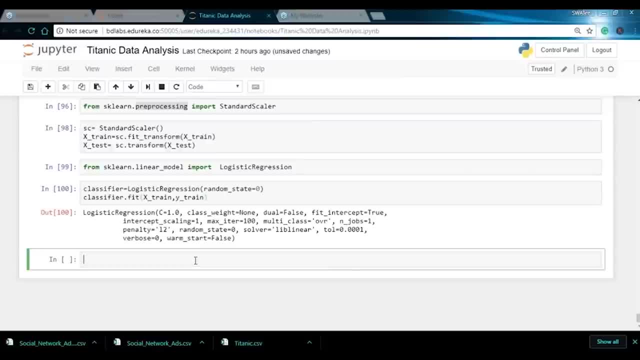 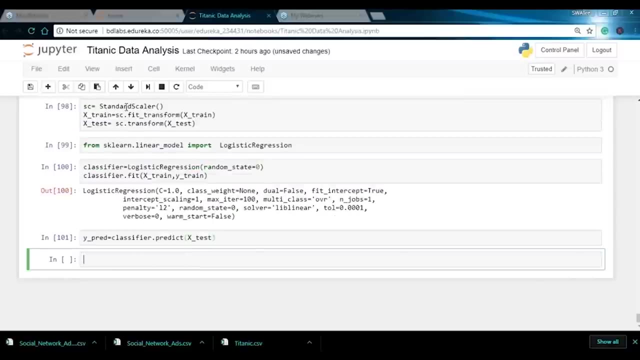 So here it tells me all the details of logistic regression. Then I have to predict the value. So I'll say wipe rate is equals to classifier, Then predict function and then I just pass in X test. So now we have created the model. 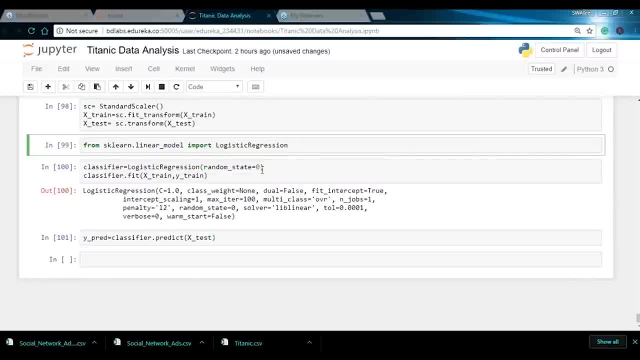 We have scaled down our input values, Then we have applied logistic Regression, we have predicted the values and now we want to know the accuracy. So to know the accuracy, first we need to import accuracy score. So I'll say: from sklearn dot metrics, import accuracy score. 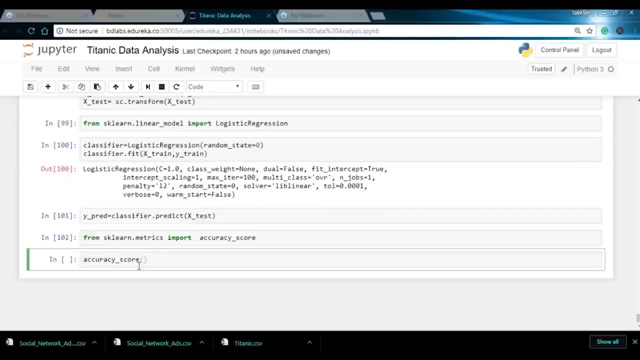 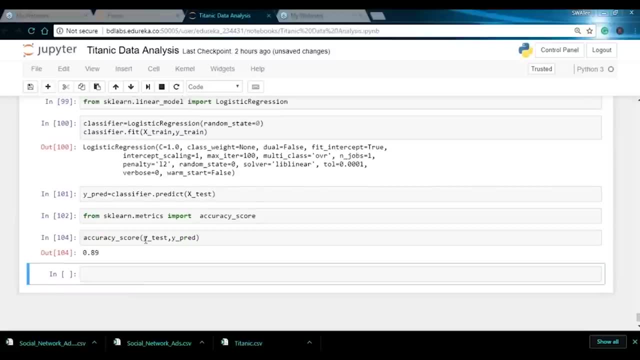 and using this function we can calculate the accuracy. or you can manually do that by creating a confusion matrix. So I just pass in my y test and my y predicted All right. So over here I get. the accuracy is 89%. so we want to know. 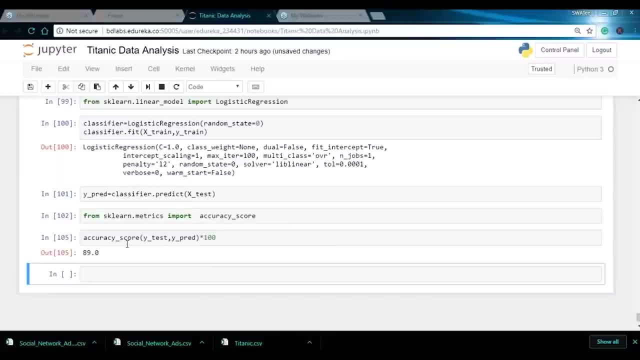 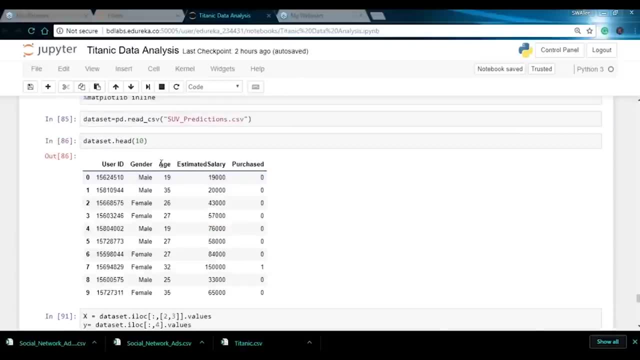 the accuracy in percentage. So I just have to multiply It by 100 and if I run this so it gives me 89%. so I hope you guys are clear with whatever I have taught you today. So here I have taken my independent variables as age and 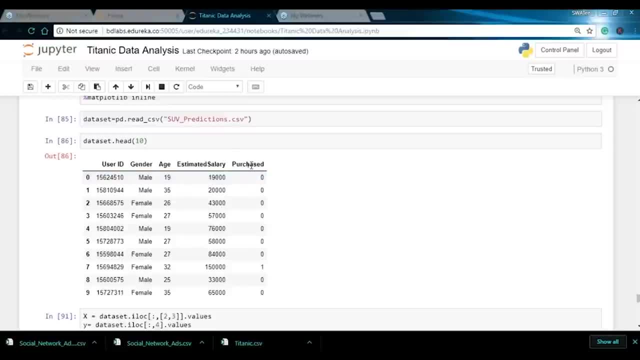 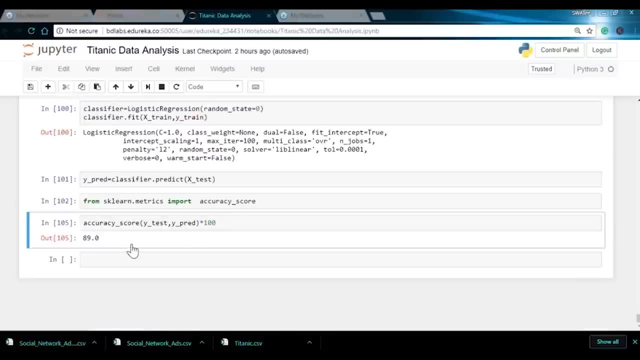 salary, and then we have calculated that- how many people can purchase the SUV. and then we have calculated our model by checking the accuracy. So over here we get, the accuracy is 89, which is great. All right, guys, that is it for today, So I'll just discuss what all we have covered in today's 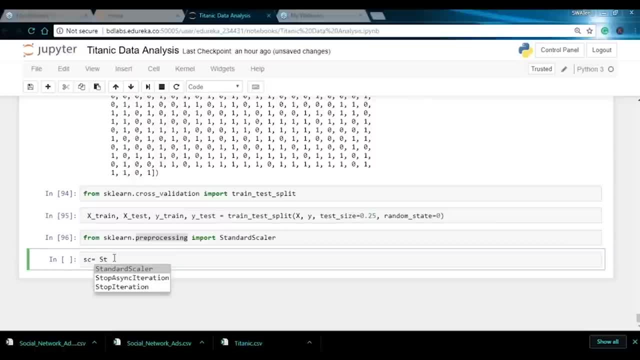 set. So I'll first make an instance of it. So I'll say standard scalar, then I'll have extreme. I'll say SC, dot, fit, fit, underscore, transform, I'll pass in my extreme variable. And similarly I can do it for test, where in I'll pass the X test. 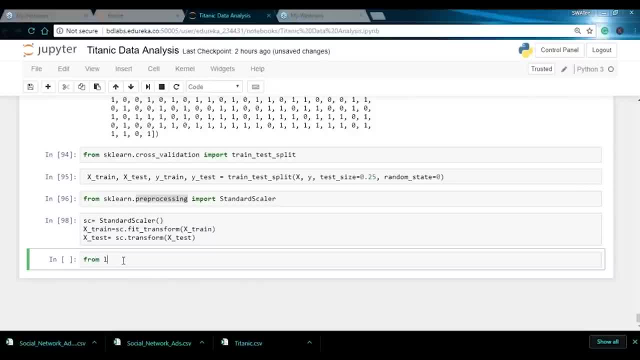 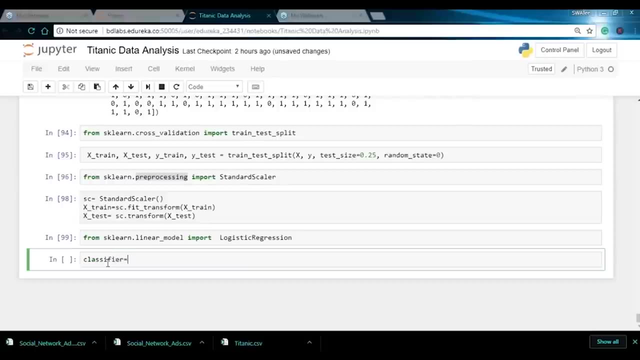 Now my next step is to import logistic regression. So I'll simply apply logistic regression by first importing it. So I'll say: from sklearn, sklearn dot linear model, import logistic regression. Over here I'll be using classifier, So I'll say: classifier dot is equals to logistic regression. 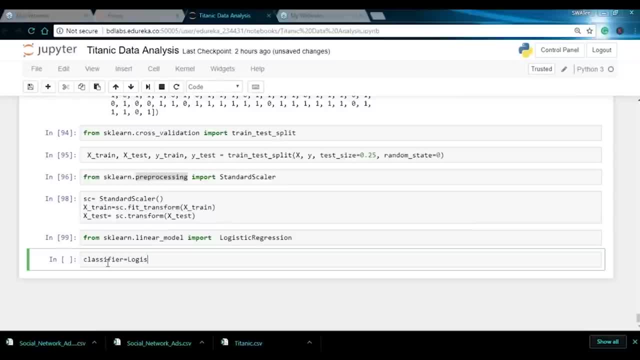 So over here I just make an instance of it. So I'll say logistic regression, and over here I just pass in the random state which is zero, And now I'll simply fit the model And I simply pass in extreme and y-train. 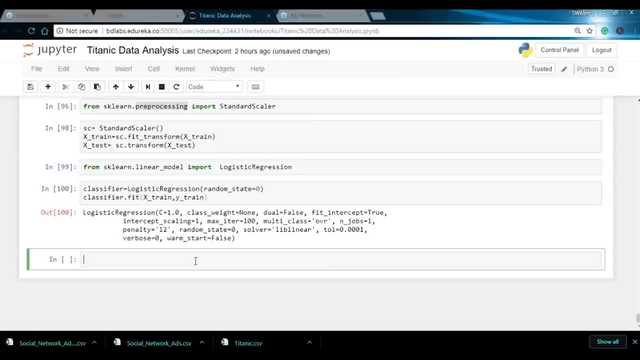 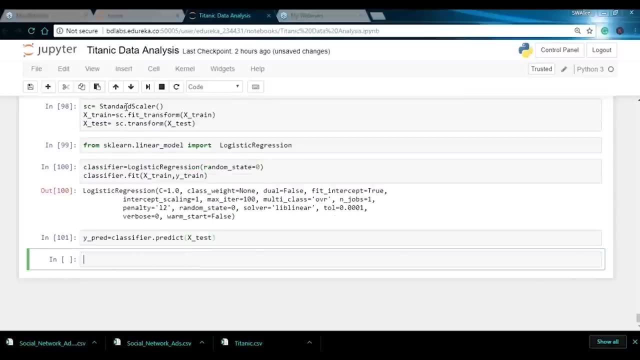 So here it tells me all the details of logistic regression. Then I have to Predict the value. So I'll say y-train, it's equals to classifier, Then predict function, and then I just pass in X test. So now we have created the model. 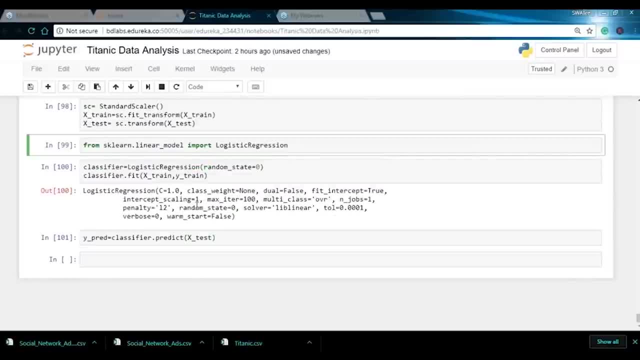 We have scaled down our input values, Then we have applied logistic regression, We have predicted the values and now we want to know the accuracy. So to know the accuracy, first we need to import accuracy score. So I'll say, from sklearn dot metrics, import accuracy score and using 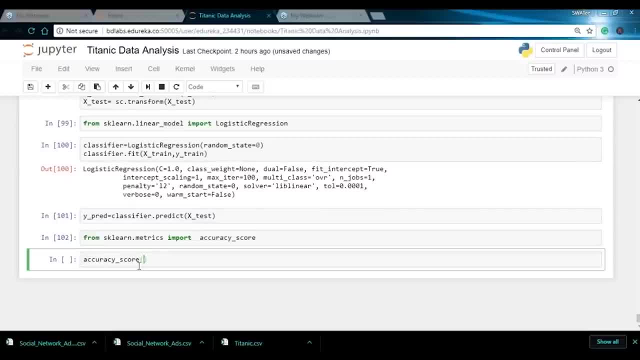 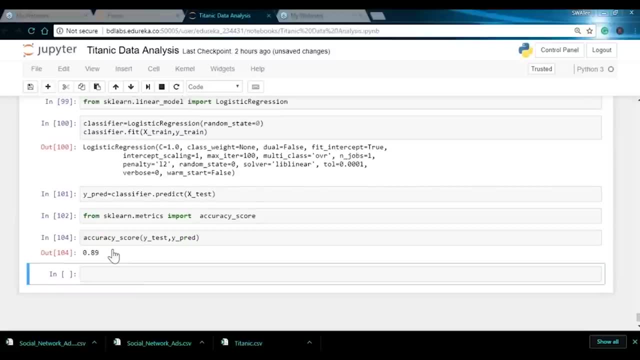 this function, We can calculate the accuracy, Or you can manually do that by creating a confusion matrix. So I just pass in my y test and my y predicted All right. so over here I get. the accuracy is 89%. so we want to know. 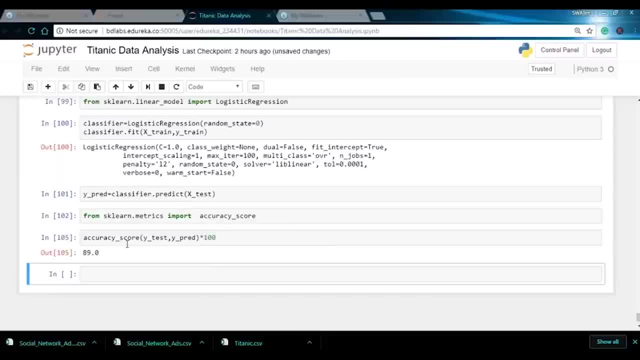 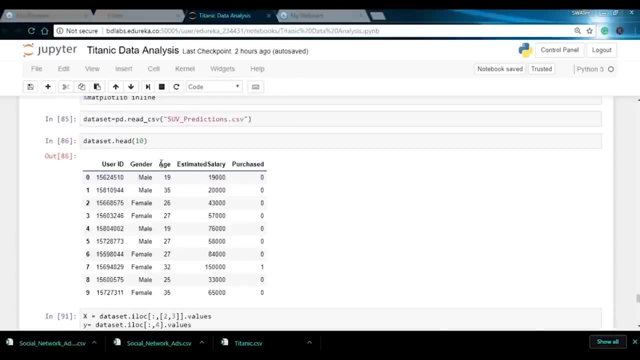 the accuracy in percentage. So I just have to multiply it by 100 and if I run this so it gives me 89%. so I hope you guys are clear with whatever I have taught you today. So here I have taken my independent variables as age and salary. 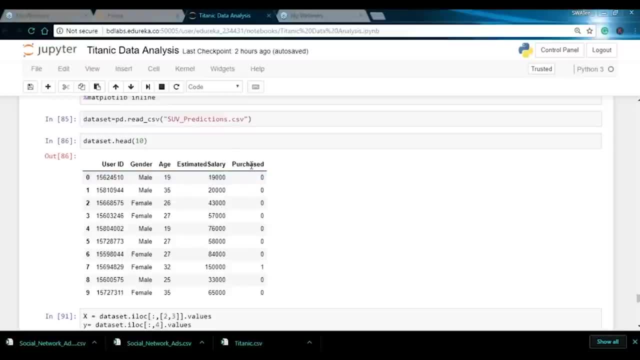 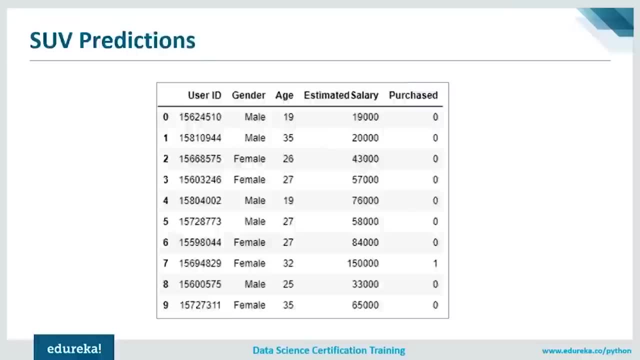 and then we have calculated that- how many people can purchase the SUV, And then we have calculated our model by checking the accuracy. So over here we get, the accuracy is 89, which is great. All right, guys, that is it for today, So I'll just discuss what all we have covered in today's training. 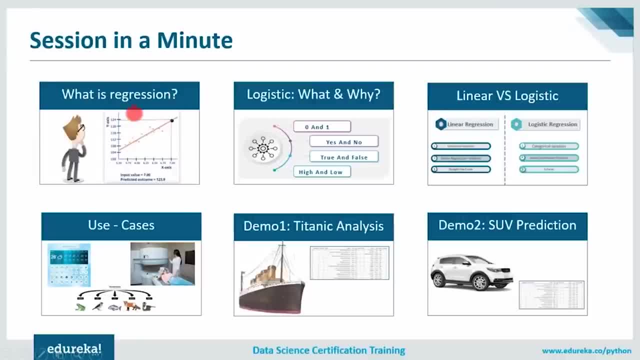 First of all, we had a quick introduction to what is regression and where the regression is actually used. then we have understood the types of regression and then got into the details of what and why of logistic regression. have compared linear versus logistic regression. We have also seen the various use cases where you can implement. 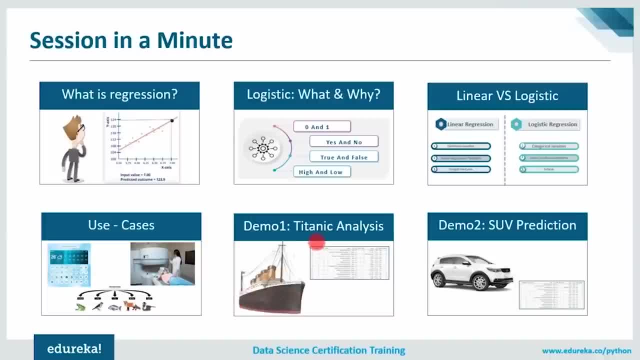 logistic regression in real life. And then we have picked up two projects, that is, Titanic data analysis and SUV prediction. over here We have seen how we can collect your data, analyze your data, then, before modeling on that data, train the data, test the data and then finally have calculated the accuracy. 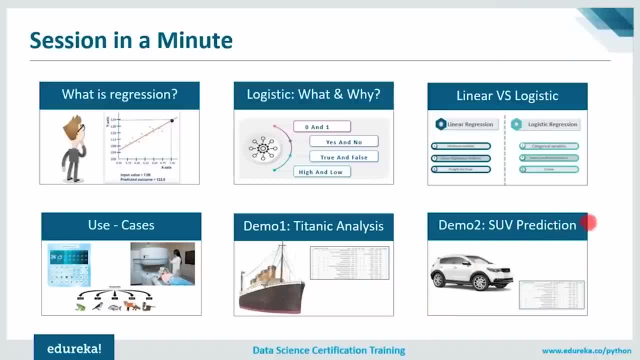 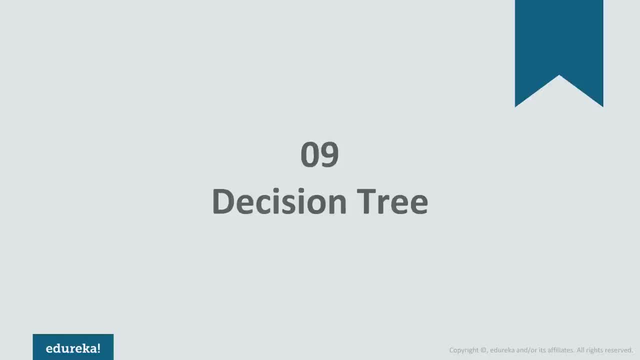 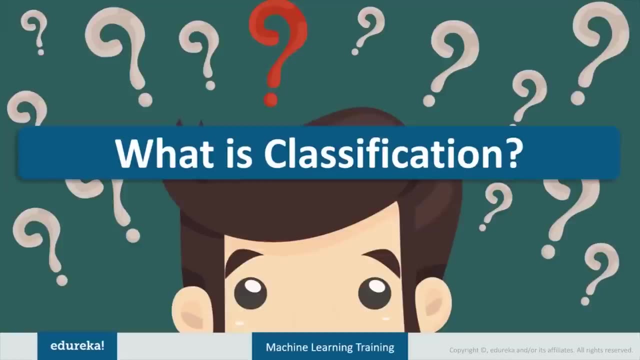 So in your SUV prediction you can actually analyze, clean your data and you can do a lot of things. so you can just go ahead, pick up any data set and explore it as much as you can. What is classification? I hope every one of you must have used Gmail. 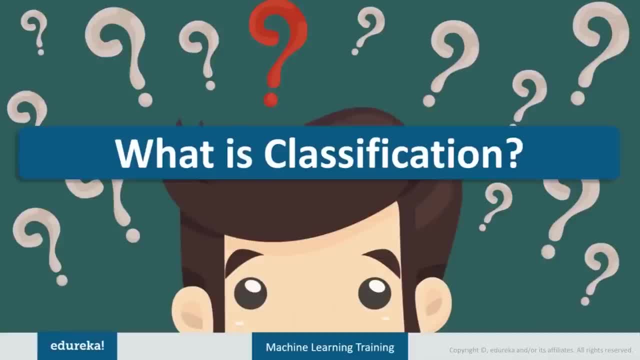 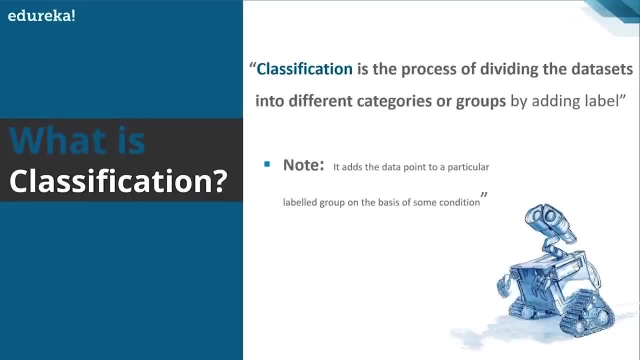 So how do you think the mail is getting classified as a spam or not a spam mail? Well, there's nothing but classification. So what it is? Well, classification is a process of dividing the data set into different categories or groups by adding label in other way, 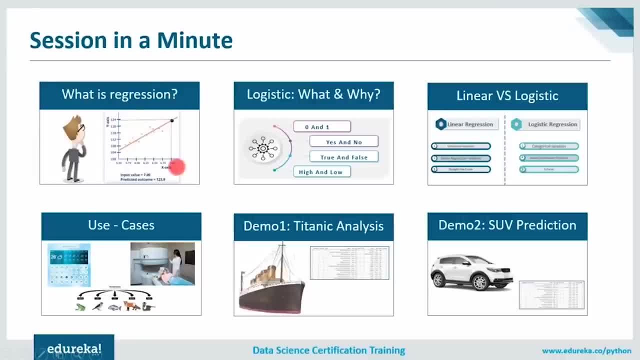 training. First of all, we had a quick introduction to what is regression and where the regression is Actually use. then we have understood the types of regression and then got into the details of what and why of logistic regression. have compared linear versus logistic regression. 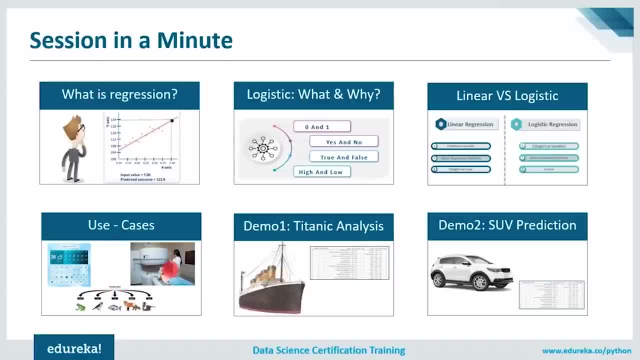 We have also seen the various use cases where you can implement logistic regression in real life. And then we have picked up two projects, that is, titanic data analysis and SUV prediction. over here We have seen how you can collect your data, analyze your data, then, before modeling on that data, train the data, test the data. 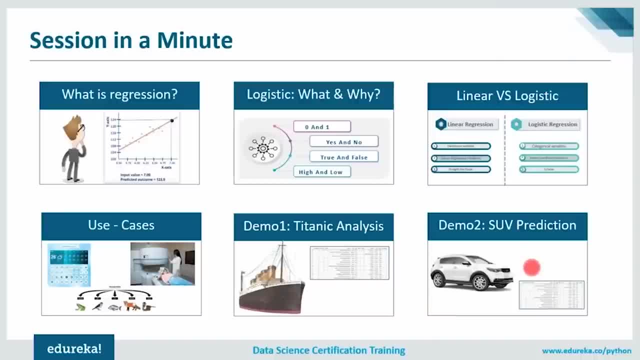 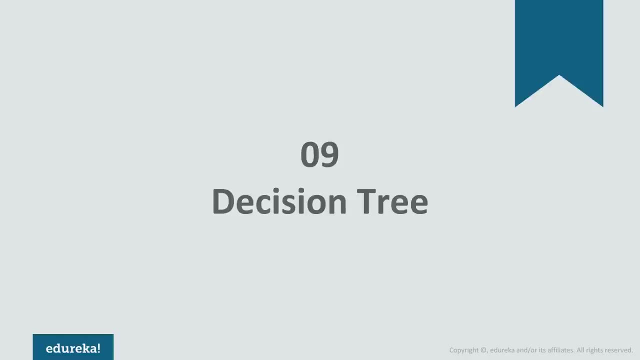 and then finally have calculated the accuracy. So in your SUV prediction you can actually analyze, clean your data and you can do a lot of things. so you can just go ahead, pick up any data set and explore it as much as you can. What is classification? 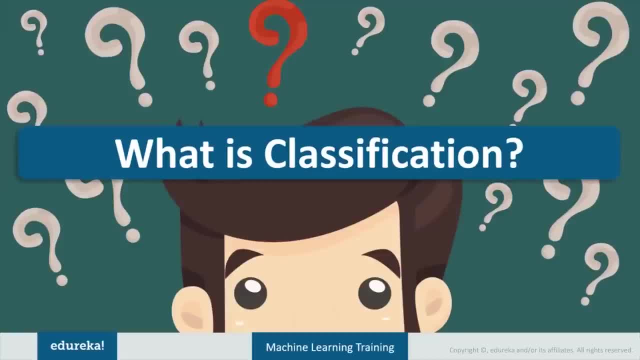 I hope every one of you must have used Gmail. So how do you think the mail is getting classified as a spam or not a spam mail? Well, there's nothing but classification. So what it is? well, classification is a process of dividing the data set into different categories or groups by adding 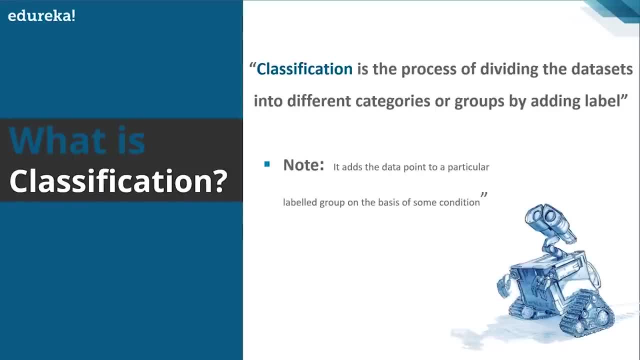 label. in other way, You can say that it is a technique of categorizing the observation into different category. So, basically, what you're doing is you're taking the data, analyzing it and, on the basis of some condition, you finally divided into various categories. Now, why do we classify it? 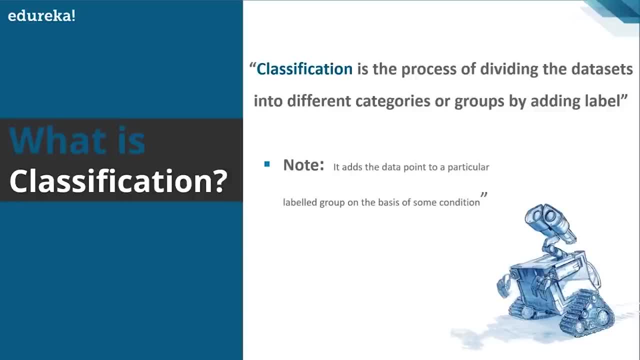 Well, we classify it to perform predictive analysis on it. Like, when you get the mail, the machine predicts it to be a spam or not a spam, a, and on the basis of that prediction it add the irrelevant Spam mail to the respective folder. in general, this classification: 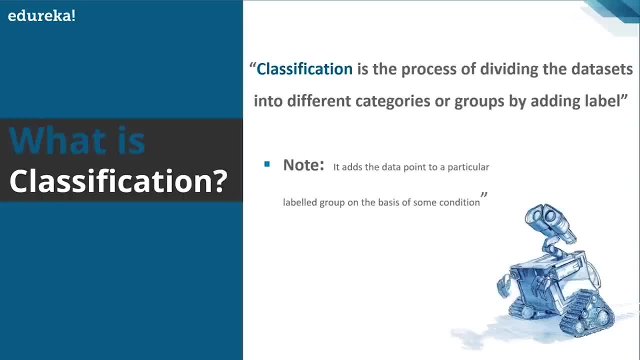 algorithm handled questions like: is this data belongs to a category or a B category, like: is this a male or is this a female, something like that. Are you getting it Okay? fine, Now the question arises: where will you use it? Well, you can use this for fraud detection or to check whether 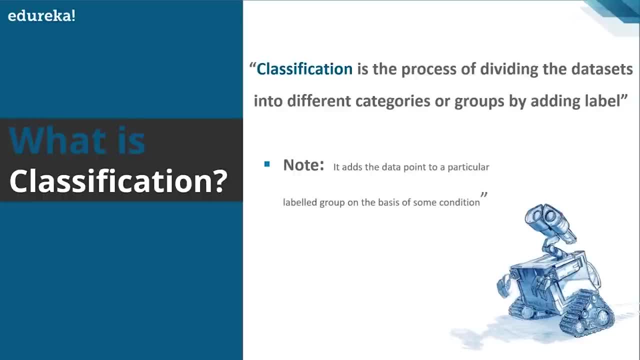 the transaction is genuine or not. Suppose I'm using a credit card here in India. now, due to some reason, I had to fly to Dubai. Now, If I'm using Credit card over there, I'll get a notification alert regarding my transaction. 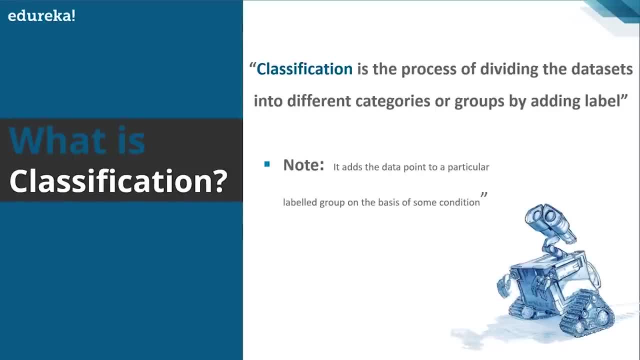 You can say that it is a technique of categorizing the observation into different category. So, basically, what you're doing Is you're taking the data, analyzing it and, on the basis of some condition, you finally divided into various categories. Now, why do we classify it? 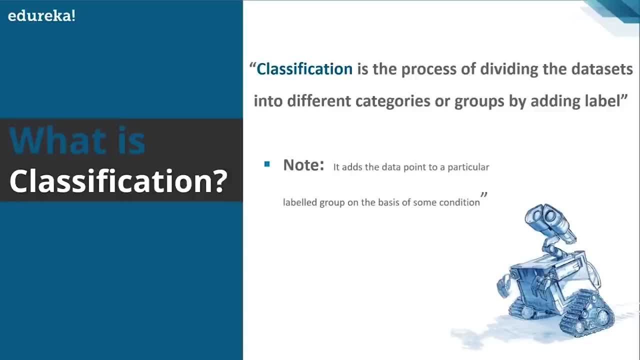 Well, we classify it to perform predictive analysis on it. Like, when you get the mail, the machine predicts it to be a spam or not a spam mail and on the basis of that prediction, it add the irrelevant or spam mail to the respective folder. in general, 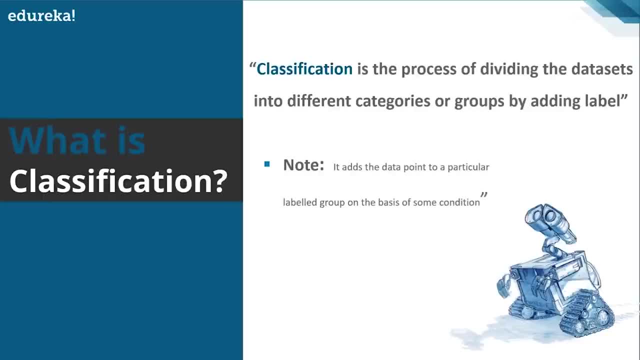 this classification algorithm handled questions like: is this data belongs to a category or B category, like: is this a mail Or is this a female? something like that? Are you getting it Okay? fine, Now the question arises: where will you use it? Well, you can use this for fraud detection or to check whether 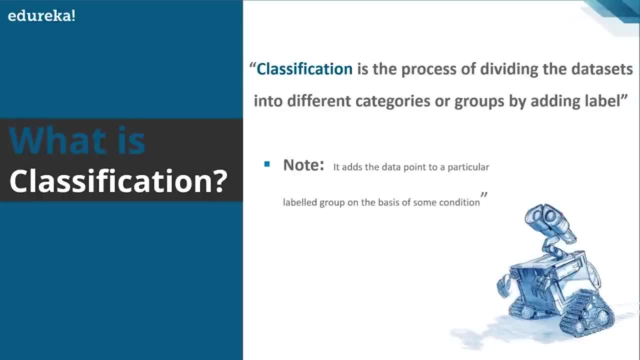 the transaction is genuine or not. Suppose I'm using a credit card here in India. now, due to some reason, I had to fly to Dubai. Now, if I'm using the credit card over there, I'll get a notification alert regarding my transaction. They would ask me to confirm about the transaction. 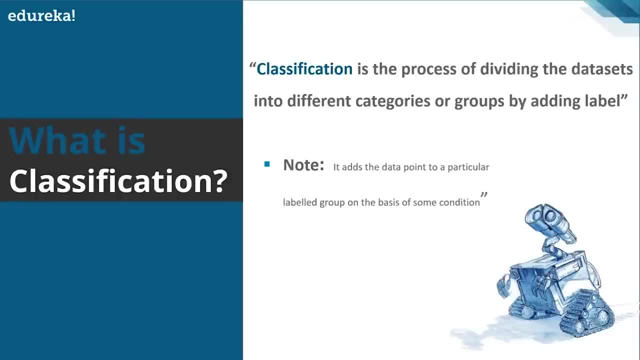 So there's also kind of predictive analysis. The machine predicts that something fishy is in the transaction, as very four hour ago I made the transaction using the same credit card in India and 24 hour later The same credit card is being used for the payment in Dubai. 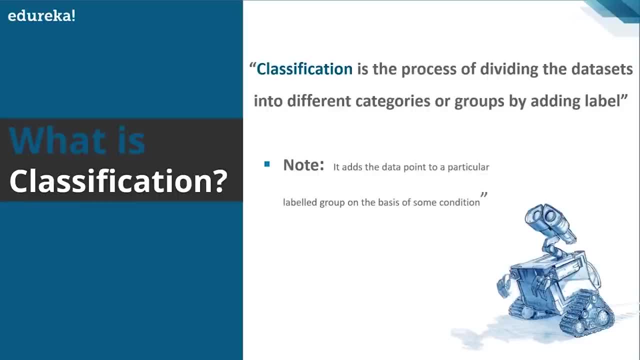 So the machine predicts that something fishy is going on in the transaction, So, in order to confirm it, it sends you a notification alert. All right, Well, this is one of the use case of classification. you can even use it to classify different items, like fruits, on the basis. 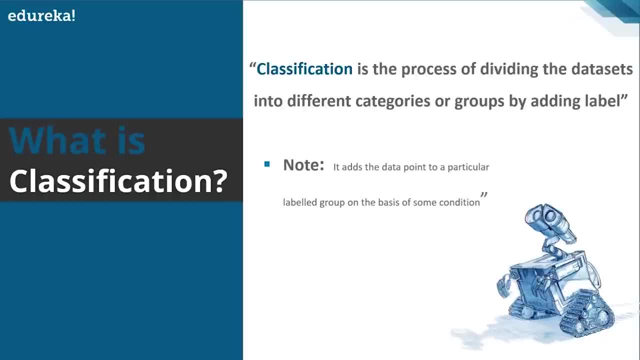 of its taste, color, Size or weight. a machine well trained using the classification algorithm can easily predict the class or the type of fruit whenever new data is given to it. Not just the fruit, It can be any item, It can be a car. 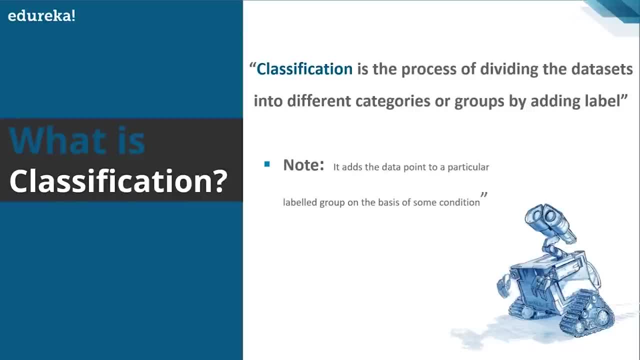 It can be a house, It can be a sign board or anything. Have you noticed that while you visit some sites or you try to log in into some, you get a picture capture for that right where you have to identify for the given images of a car or it's of a? 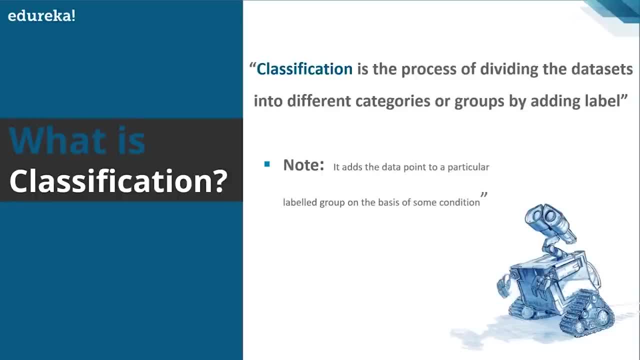 They would ask me to confirm about the transaction. So there's also kind of predictive analysis, as the machine predicts that something fishy is in the transaction, as very four hour ago I made the transaction using the same credit card in India, and 24 hour later 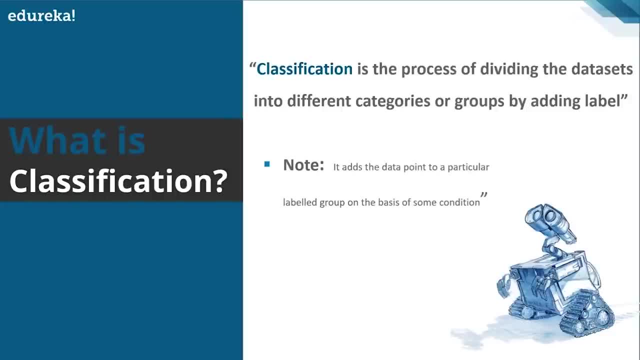 The same credit card is being used for the payment in Dubai, So the machine predicts that something fishy is going on in the transaction. So, in order to confirm it, It sends you a notification alert. All right, Well, this is one of the use case of classification. 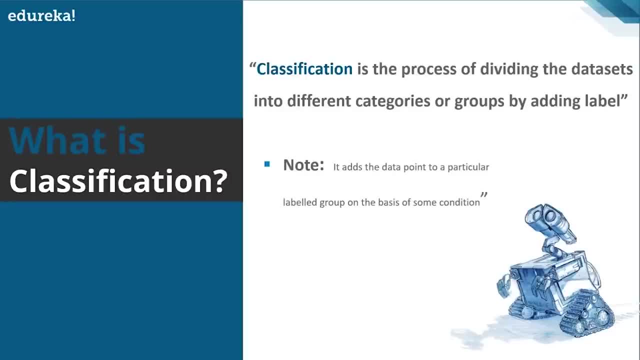 You can even use it to classify different items, like fruits, on the base of its taste, color, size or weight. a machine well trained using the classification algorithm can easily predict the class or the type of fruit whenever new data is given to it, Not just the fruit. 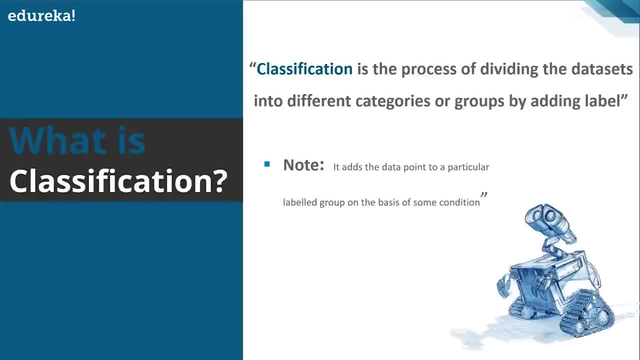 It can be any item. It can be a car, It can be a house, It can be a sign board or anything. Have you noticed that while you visit some sites or you try to login into some, you get a picture capture for that right where? 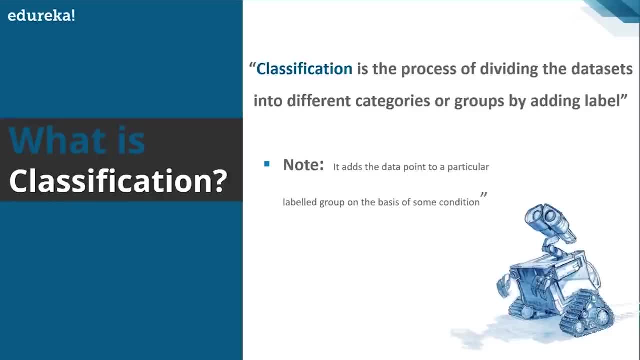 you have to identify for the given images- of a car or it's of a pole or not- You have to select it. For example, there are 10 images and you're selecting three images out of it. So in a way, you are training the machine, right. 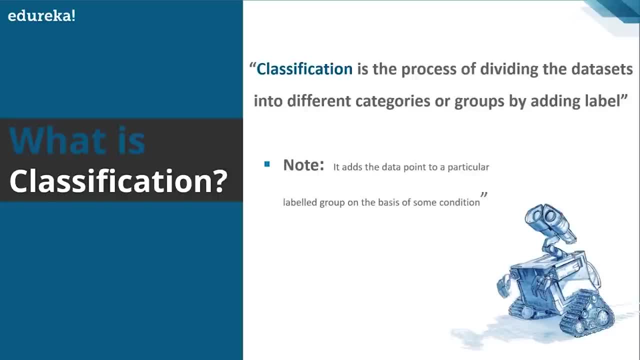 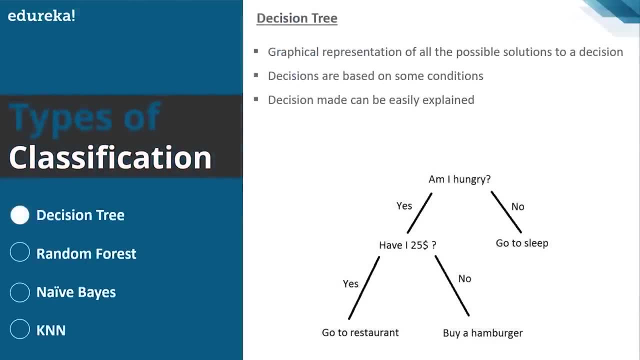 You're telling that these three are the picture of a car and rest are not, So who knows? you are training it for something big, right? So, moving on ahead, Let's discuss the types of classification. All right? Well, there are several different ways to perform a same task. 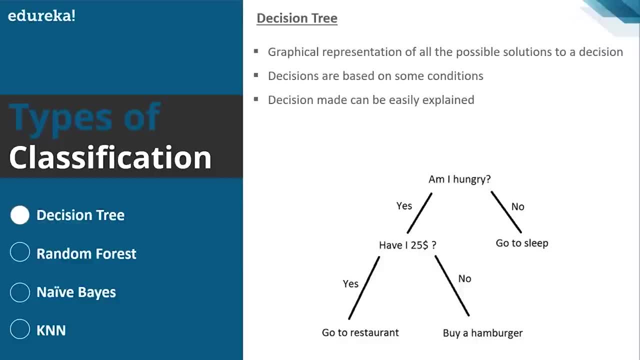 Like, in order to predict with a given person is a male or a female, the machine had to be trained first. All right, but there are multiple ways to train the machine and you can choose any one of them just for predictive analytics. There are many different techniques, but the most common of them 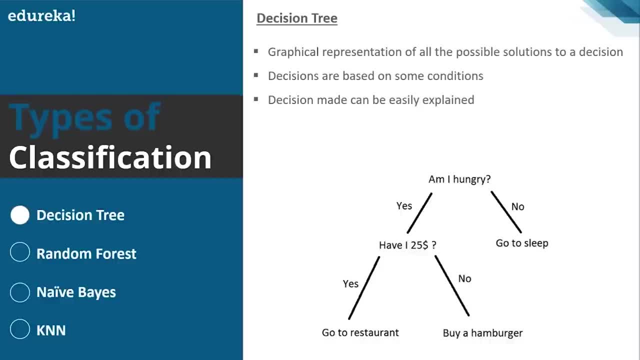 all is the decision tree, which will cover in depth in today's session. So as a part of classification algorithm, we have decision tree, random Forest, neighbors, k nearest neighbor, logistic regression, linear regression, support vector machines and so on. There are many, All right. 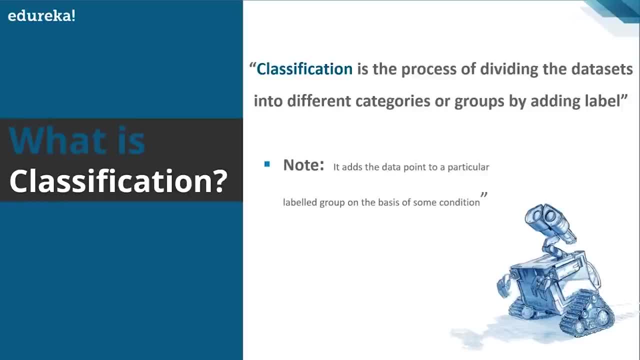 pole or not. You have to select it. For example, there are 10 images And you're selecting three images out of it. So in a way, you are training the machine right. You're telling that these three are the picture of a car and rest. 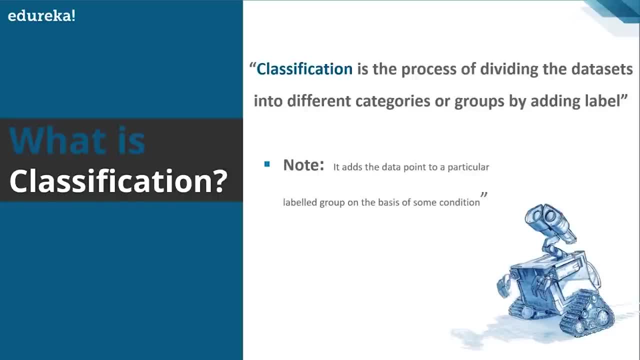 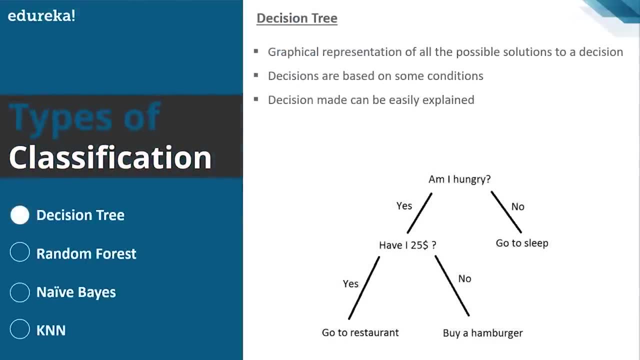 are not. So, who knows, you are training it for something big right. So, moving on ahead, Let's discuss the types of classification. All right, Well, there are several different ways to perform a same task, like in order to predict with a given person is a male or a female. the 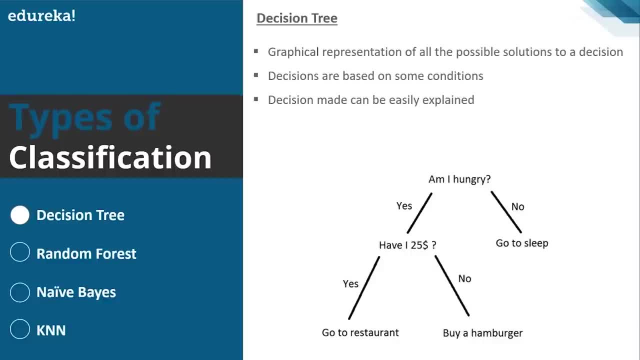 machine had to be trained first. All right, but there are multiple ways to train the machine and you can choose any one of them Just for predictive analytics. There are many different techniques, but the most common of them all is the decision tree, which will cover in depth in today's 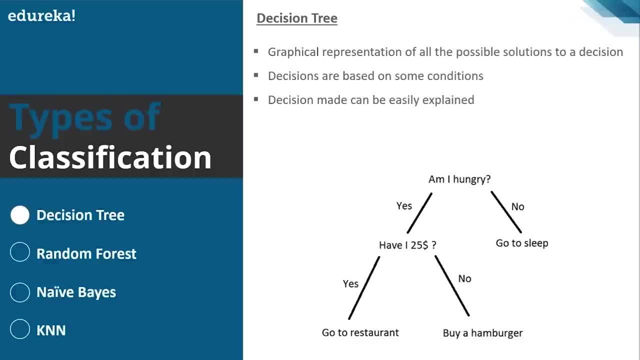 session. So, as a part of classification algorithm, we have decision tree, random Forest, neighbors, k, nearest neighbor, logistic regression, linear regression, support vector machines and so on. There are many, All right, So let me give you an idea about few of them, starting with 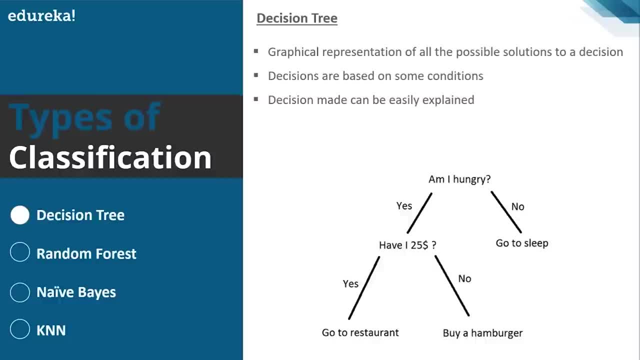 decision tree. A decision tree is a graphical representation of all the possible solution to a decision, The decisions Which are made. they can be explained very easily. For example, here is a task which says that should I go to a restaurant or should I buy a hamburger? 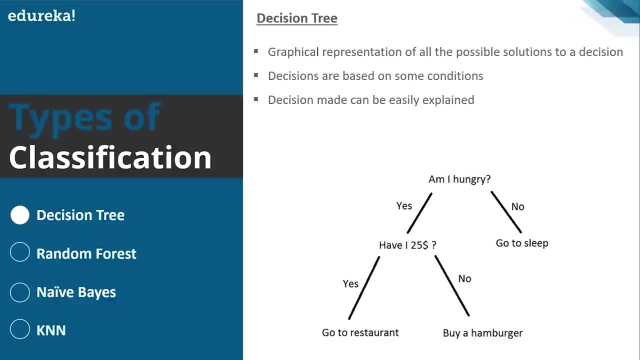 You are confused on that. So, for that, what you will do will create a decision tree for it. starting with the root node will be: first of all, you'll check whether you are hungry or not. All right, if you're not hungry, then just go back to sleep, right? 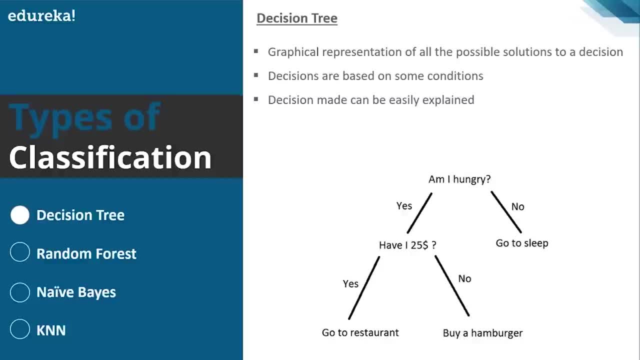 If you are hungry and you have $25, then you will decide to go to restaurant, and if you're hungry and you don't have $25, then you'll just go and buy a hamburger. That's it, All right. So this is about decision tree. 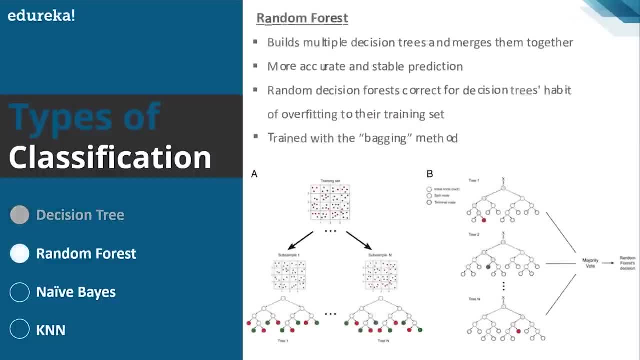 Now moving on ahead. Let's see What is a random Forest. will random Forest build multiple decision trees and merges them together to get a more accurate and stable prediction. All right, most of the time, random Forest is trained with a bagging method. 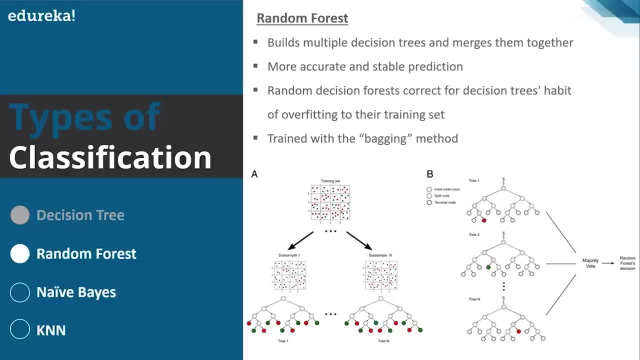 The bagging method is based on the idea that the combination of learning model increases the overall result. if you are combining the learning from different models And then clubbing it together, what it will do? It will increase the overall result, fine. Just one more thing: if the size of your data set is huge, then in that 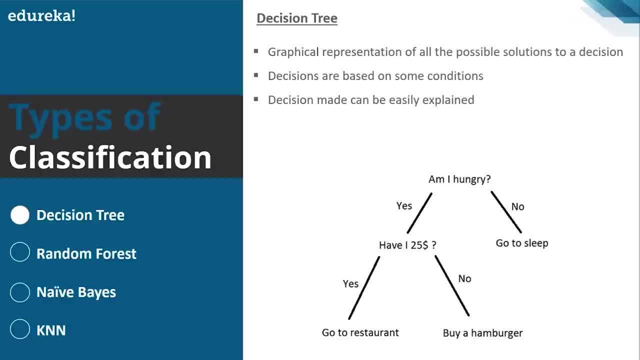 So let me give you an idea about few of them, starting with decision tree. Well, decision tree is a graphical representation of all the possible solution to a decision, the decisions which are made. They can be explained very easily. For example, here is a task which says that should I go to a restaurant? 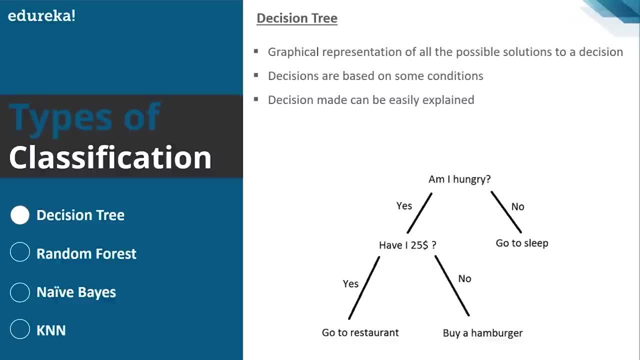 or should I buy a hamburger? You are confused on that. So for that, what you will do will create a decision tree for it, starting with the root node, will be: first of all, you'll check whether you are hungry or not. All right if you're not hungry. 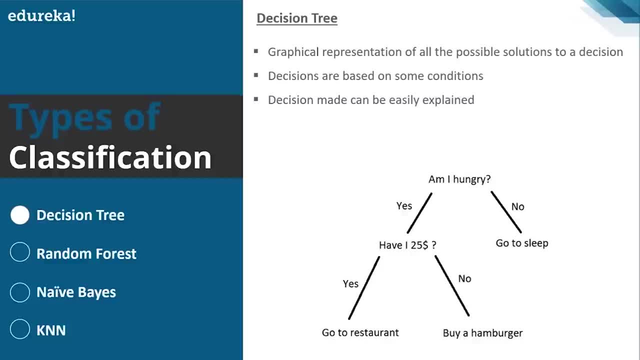 Then just go back to sleep, right? If you are hungry and you have $25, then you will decide to go to restaurant, and if you're hungry and you don't have $25, then you'll just go and buy a hamburger. That's it. 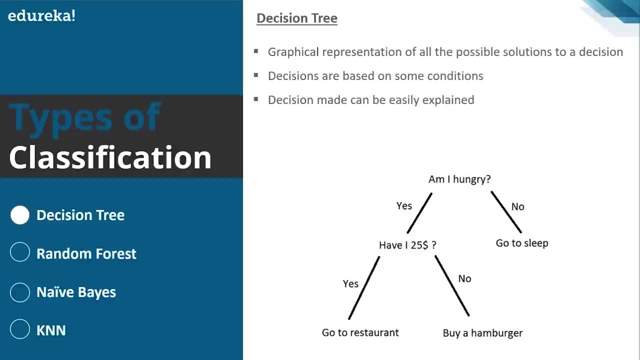 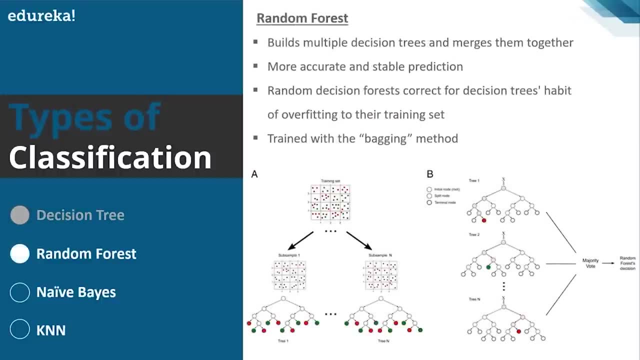 All right, So this is about decision tree. now, moving on ahead, Let's see What is a random Forest. will random Forest build multiple decision trees and merges them together to get a more accurate and stable prediction? All right, most of the time, random Forest is trained with a. 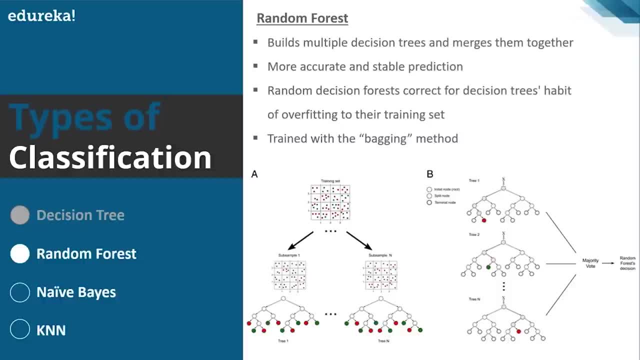 bagging method. The bagging method is based on the idea that the combination of learning model increases the overall result. If you are combining the learning from different models and then clubbing it together, what it will do? it will increase the overall result. Fine. 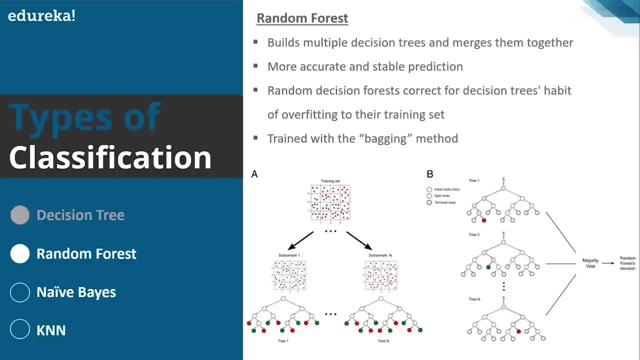 Just one more thing. if the size of your data set is huge, then in that case one single decision tree would lead to a overfit model, same way, like a single person might have its own perspective on the complete population, as a population is very huge, right. 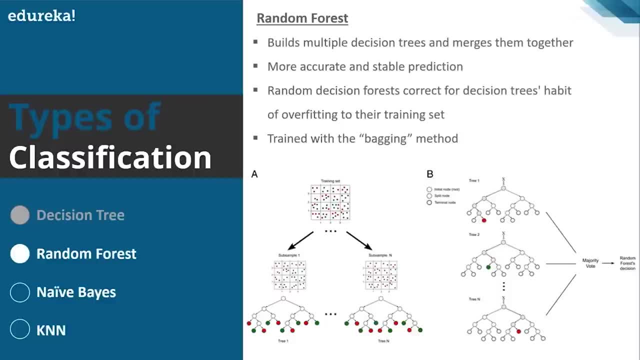 However, if we implement the voting system and ask different individual to interpret the data, then we would be able to cover the pattern in a much meticulous way. even from the diagram You can see that in section a we have a large training data set- what we do. 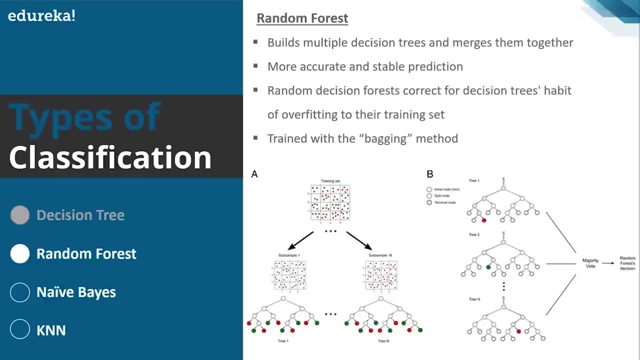 We first divide our training data set into n sub samples- All right- and we create a decision tree for each sub sample. now, in the B part, what we do? we take the vote out of every decision made by every decision tree and finally, we club the vote to get. 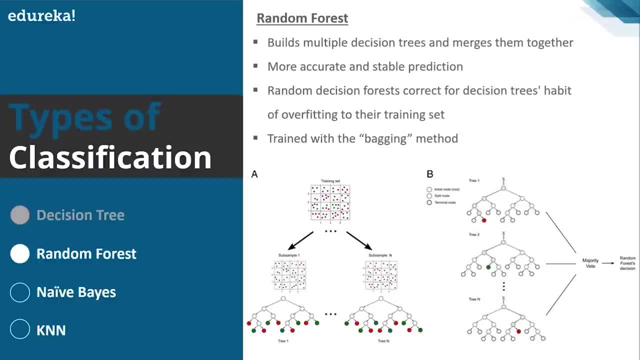 case, one single decision tree would lead to a overfit model, same way, like a single person might have its own perspective on the complete population, as a population is very huge right. However, if we implement the voting system and ask different individual to interpret the data, then we would be able to cover the pattern in a 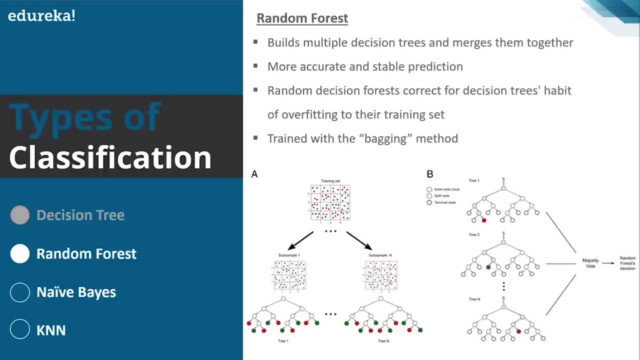 much meticulous way. Even from the diagram you can see that in section a we have a large training data set. what we do? we first divide our training data set into n sub samples, All right, and we create a decision tree for each sub sample. now in 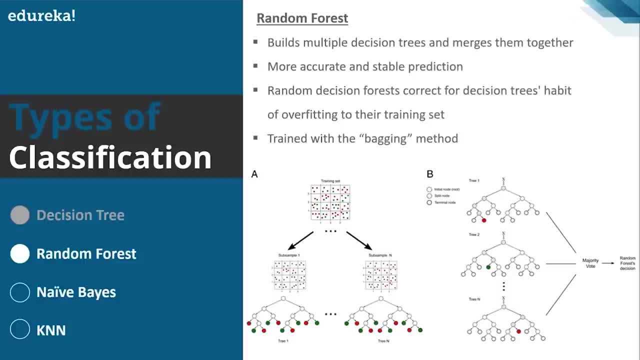 the B part, what we do. we take the vote out of every decision made by every decision tree And finally we club the vote to get the random Forest decision. fine, Let's move on ahead. Next we have nape bias. So nape bias is a classification. 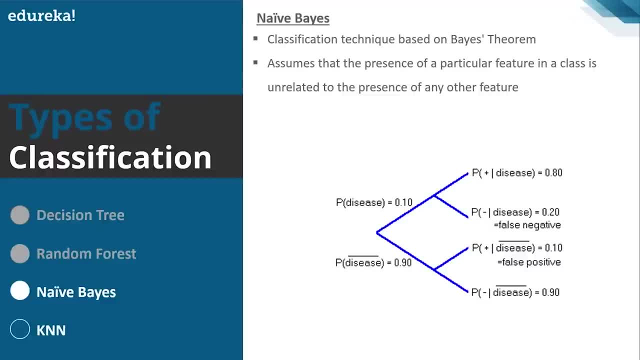 Technique which is based on Bayes theorem. It assumes that presence of any particular feature in a class is completely unrelated to the presence of any other feature. nape bias is simple and easy to implement algorithm and, due to a simplicity, this algorithm might outperform more complex model when the size of 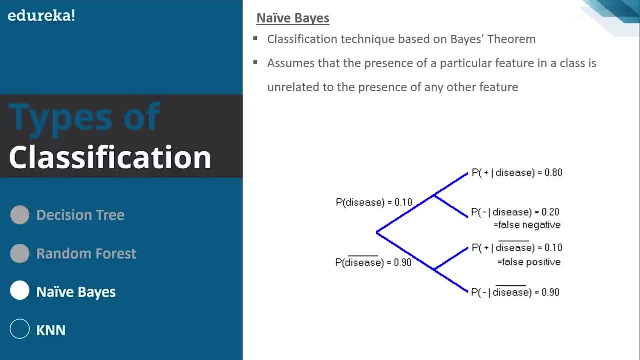 the data set is not large enough, All right. a classical use case of nape bias is a document classification. and that what you do? you determine whether given text corresponds to one or more categories. In the text case, the features used might be the presence or absence. 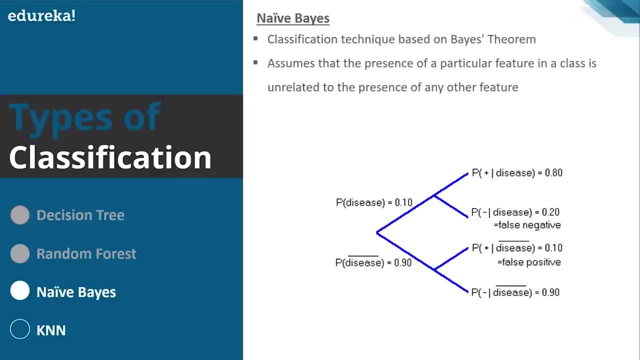 of any keyword, So this was about name. from the diagram You can see that using nape bias We have to decide whether we have a disease or not first. what we do, we check the probability of having a disease and not having the disease right. probability of having a disease is 0.1, while on the 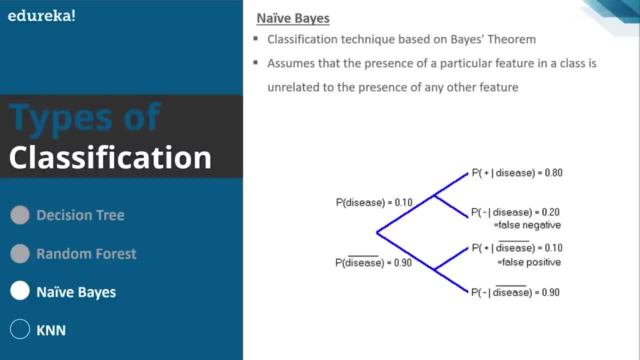 other hand, probability of not having a disease is 0.9.. Okay, First let's see when we have disease and we go to doctor. Are they so when you visited the doctor and the test is positive, so probability of having a positive test when you're having a disease is. 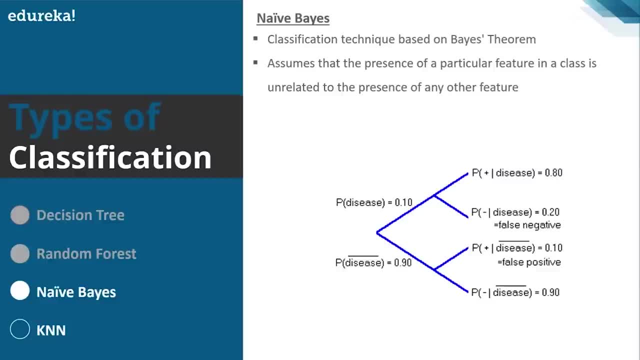 0.80 and probability of a negative test when you already have a disease that is 0.20.. This is also a false negative statement as the test is detecting negative, but you still have the disease right. So it's a false negative statement. 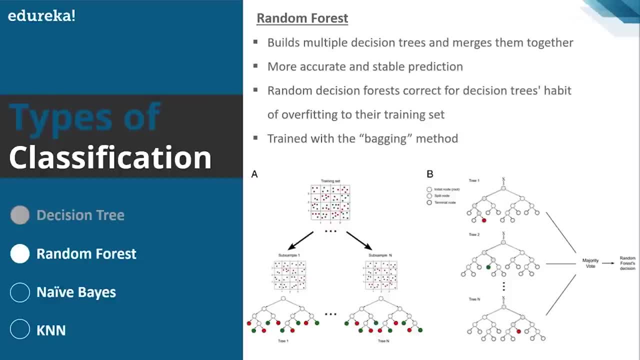 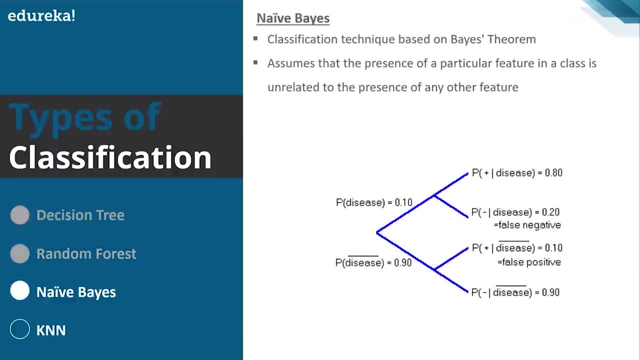 the random forest decision. fine, Let's move on ahead. Next we have nabias. So nabias is a classification technique which is based on Bayes theorem. It assumes that presence of any particular feature in a class is completely unrelated to the presence of any other feature. 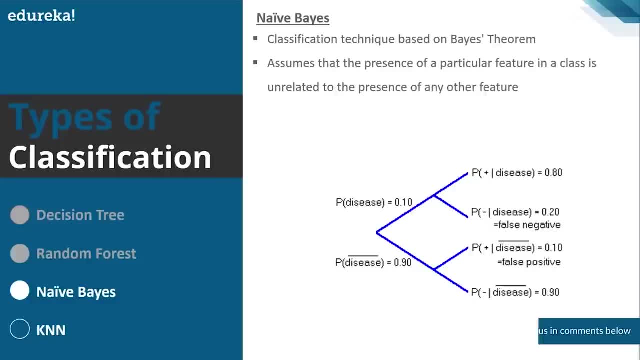 nabias is simple and easy to implement algorithm and due to its simplicity, this algorithm might outperform more complex model when the size of the data set is not large enough. All right, a classical use case of nabias is a document classification. and that what you do? you determine whether given text corresponds. 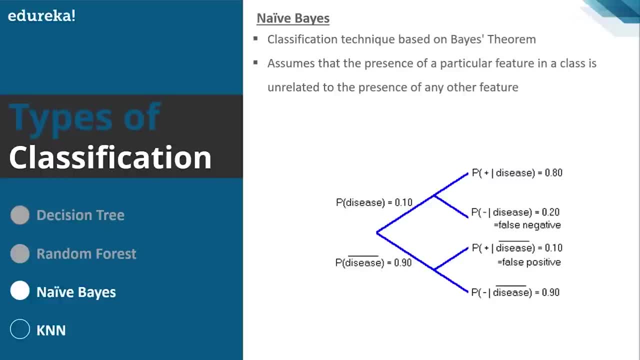 to one or more categories. in the text case, the features used might be the presence or absence of any keyword, So this was about name. from the diagram You can see that using nabias, We have to decide whether we have a disease or not first what we 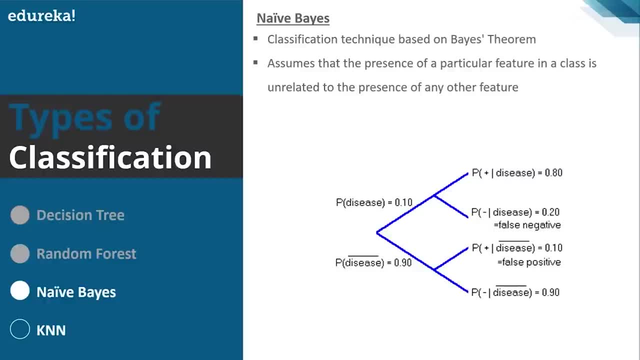 do we check the probability of having a disease and not having the disease? right, probability of having a disease is zero- 0.1- while on the other hand, probability of not having a disease is 0.9.. Okay, First let's see when we have disease and we go to doctor early. 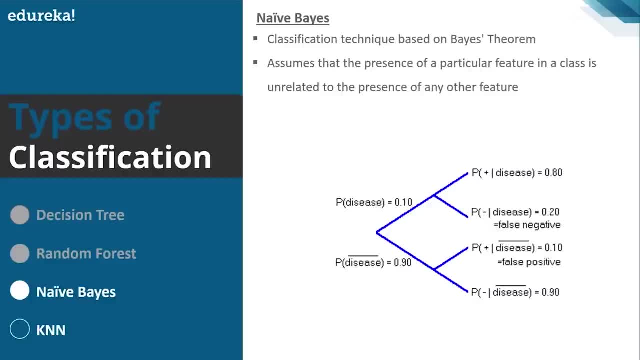 So when you visited the doctor and the test is positive, so probability of having a positive test when you're having a disease is 0.80 and probability of a negative test when you already have a disease that is 0.20.. This is also a false negative statement, as the test is detecting. 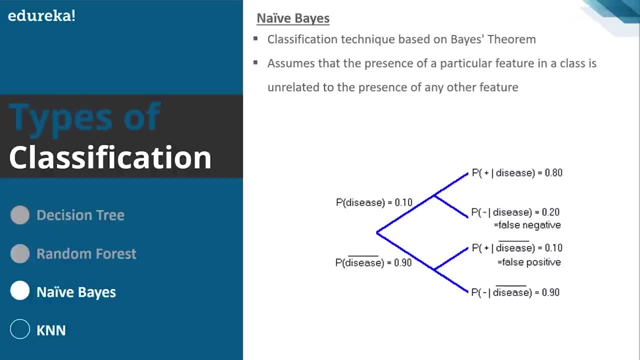 negative, But you still have the disease right. So it's a false negative statement. Now let's move ahead when you don't have the disease at all. So probability of not having a disease is 0.9, and when you visit, 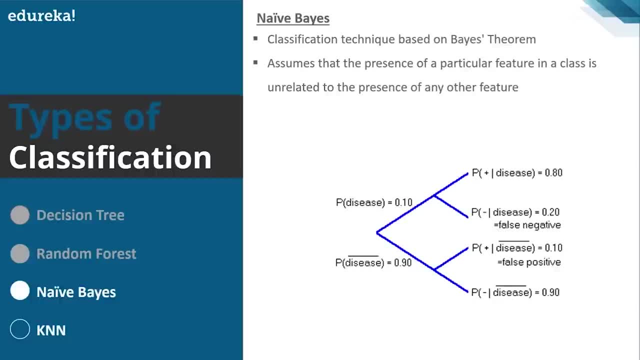 the doctor and the doctor is like: yes, you have the disease, but you already know that you don't have the disease. So it's a false positive statement. So probability of having a disease when you actually know there is no disease is 0.1, and probability of not having a disease 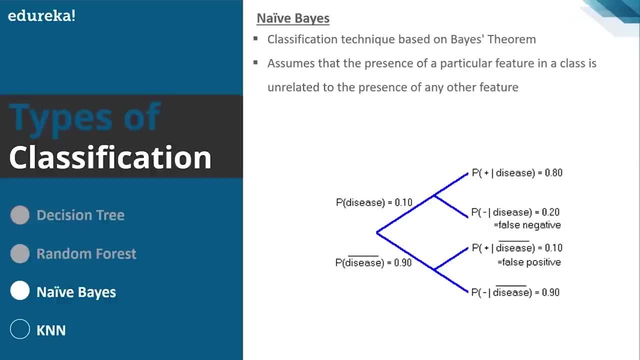 when you actually know there is no disease. so, and the probability it is around 0.90, fine, it is same as probability of not having a disease. even the test is showing the same result. it's a true positive statement. so it is 0.9, all right, so let's move on ahead. 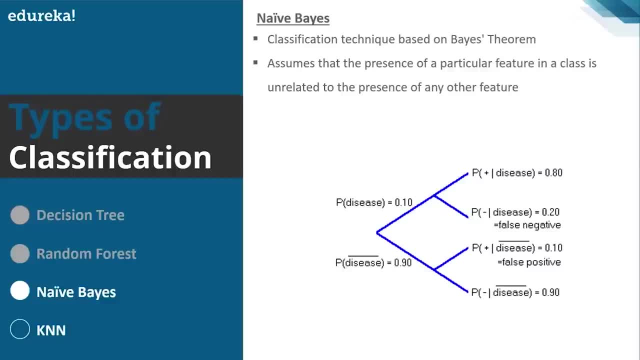 Now let's move ahead when you don't have the disease at all. So probability of not having a disease is 0.9.. And when you visit the doctor and the doctor is like, yes, you have the disease, but you already know that you don't have the disease, 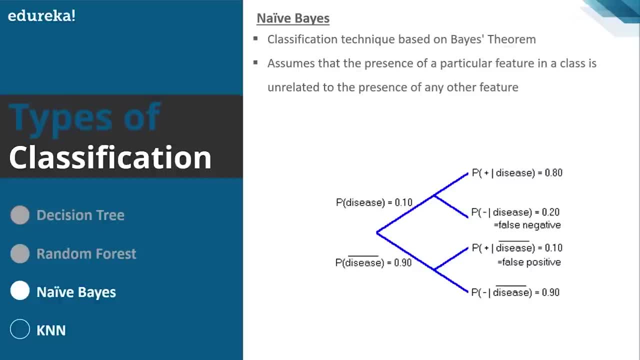 So it's a false positive statement. So probability of having a disease when you actually know there is no disease is 0.1, and probability of not having a disease when you actually know there is no disease. So and the probability of it is around 0.90. fine, 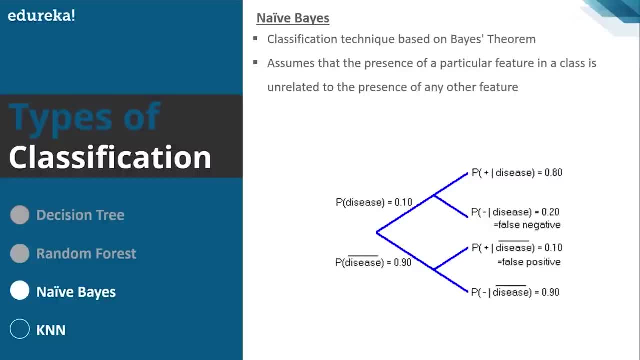 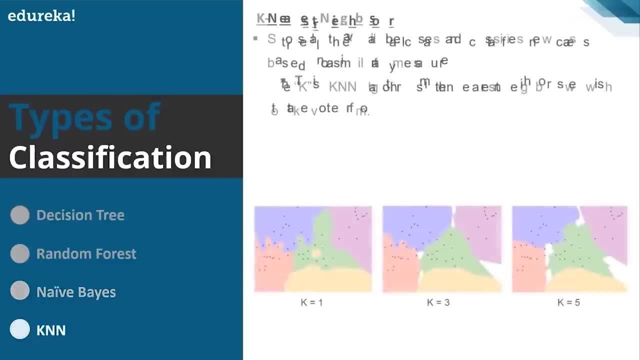 It is same as probability of not having a disease. in the test is showing the same result, the true positive statement. So it is 0.9.. All right, So let's move on ahead and discuss about K&N algorithm. So this K&N algorithm or the K nearest neighbor? 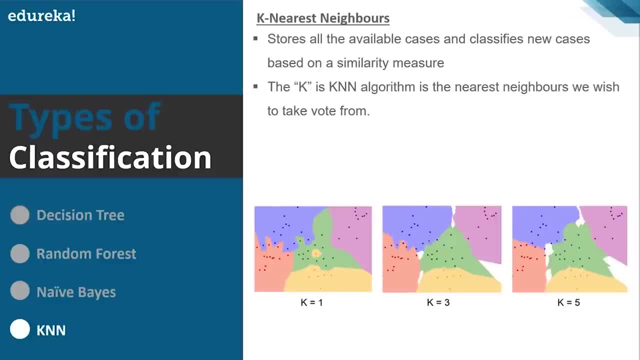 It stores all the available cases and classifies new cases based on the similarity measure. The K in the K&N algorithm is the nearest neighbor we wish to take vote from. For example, if K equal 1,, then the object is simply assigned. 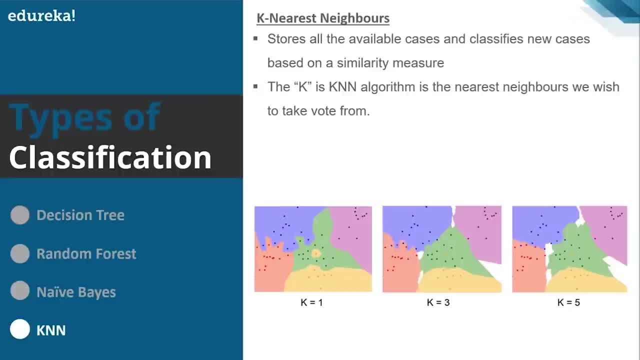 to the class of that single nearest neighbor. from the diagram You can see the difference in the image when K equal 1, K equal 3 and K equal 5, right Well, the modern systems are now able to use the K nearest neighbor. 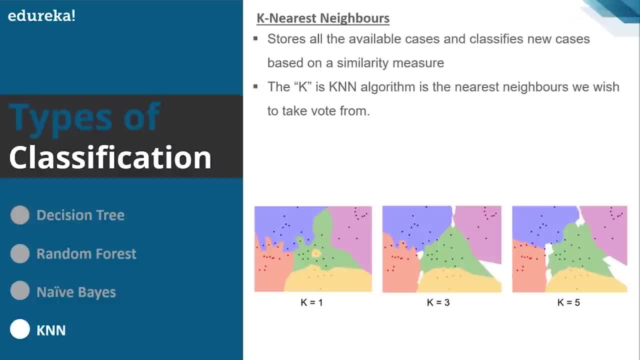 for visual pattern recognition to scan and detect hidden packages in the bottom bin of a shopping cart at the checkout. If an object is detected which matches exactly to the object listed in the database, then the price of the spotted product could even automatically be added to the customer's bill. 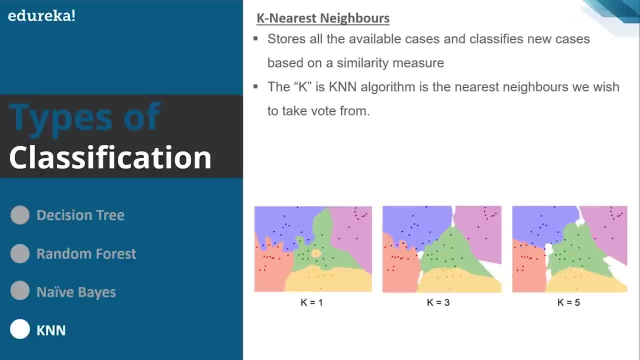 While this automated billing practice is not used extensively at this time, But the technology has been developed and is available for use. If you want, you can just use it. And yeah, one more thing: K nearest neighbor is also used in retail to detect patterns in the credit card users. 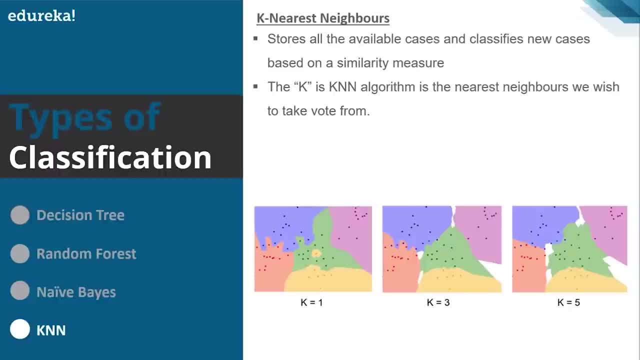 Many new transaction scrutinizing software application use K&N algorithms to analyze register data and spot unusual pattern that indicates suspicious activity. For example, if register data indicates that a lot of customers information is being entered manually rather than through automated scanning and swapping, Then in that case this could indicate that the employees who 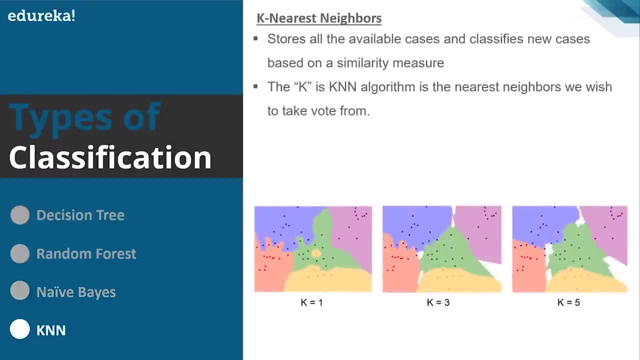 and discuss about knn algorithm. so this knn algorithm or the k nearest neighbor. it stores all the available cases and classifies new cases based on this similarity measure. the k in the knn algorithm is the nearest neighbor we wish to take vote from. for example, if k equal 1, then the 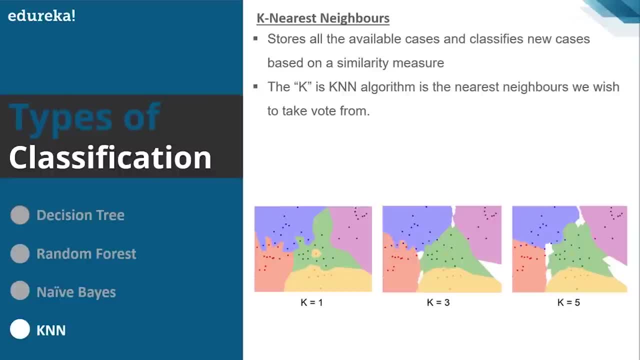 object is simply assigned to the class of that single nearest neighbor. from the diagram you can see the difference in the image when k equal 1, k equal 3 and k equal 5. right well, the modern systems are now able to use the k nearest neighbor for visual pattern recognition, to scan and detect. 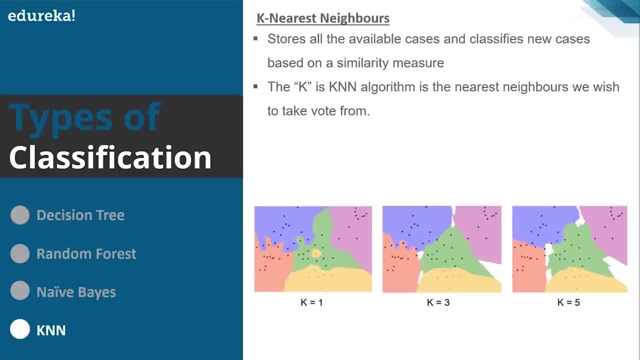 hidden packages in the bottom bin of a shopping cart. at the checkout, if an object is detected which matches exactly to the object listed in the database, then the price of the spotted product could even automatically be added to the customer's bill, while this automated billing practice is not. 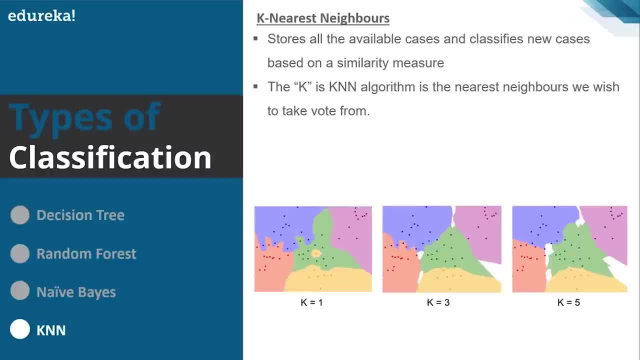 used extensively at this time, but the technology has been developed and is available for use. if you want, you can just use it. and yeah, one more thing: k nearest neighbor is also used in retail to detect patterns in the credit card users. many new transaction scrutinizing software application. 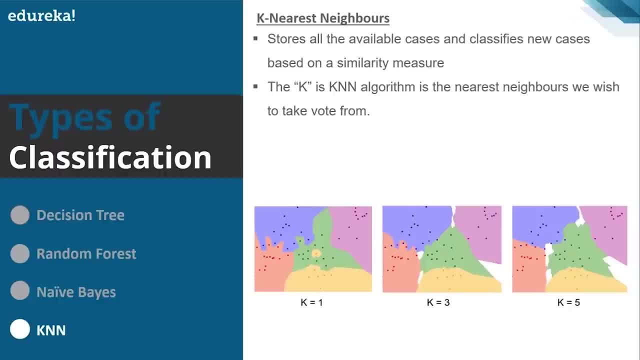 use knn algorithm to analyze registered data and spot unusual pattern that indicates suspicious activity. for example, if registered data indicates that a lot of customers information is being entered manually rather than through automated scanning and swapping, then in that case this could indicate that the employees who are using the register are in fact stealing customers personal information. 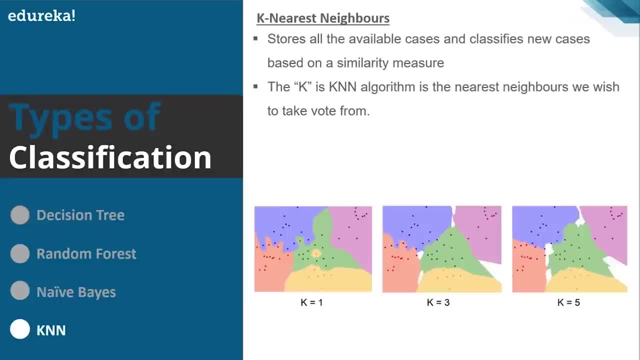 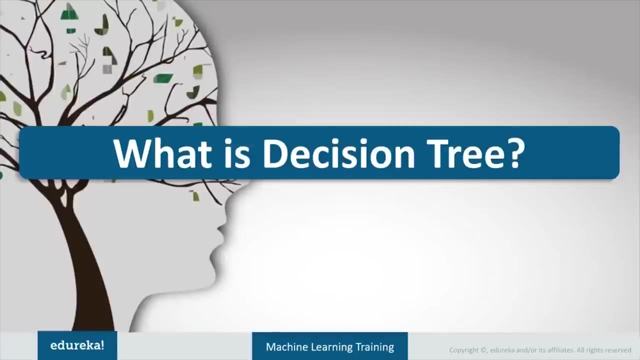 or if a registered data indicates that a particular good is being returned or exchanged multiple times. this could indicate that employees are misusing the return policy or trying to make money from doing the fake returns. right, so this was about knn algorithm. so starting with what is decision tree? but first let me tell you why did we choose. 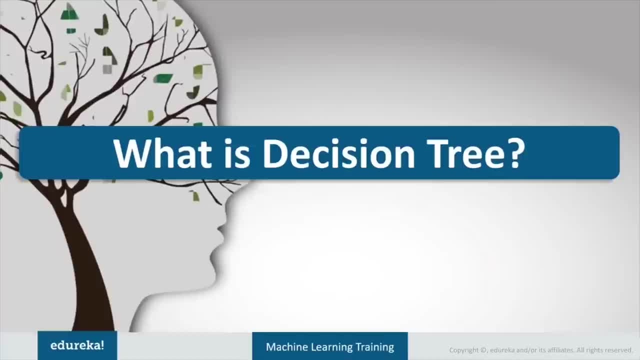 decision tree to start with. well, these decision tree are really very easy to read and understand. it belongs to one of the few models that are interpretable where you can understand exactly why the classifier has made that particular decision right. let me tell you a fact that for 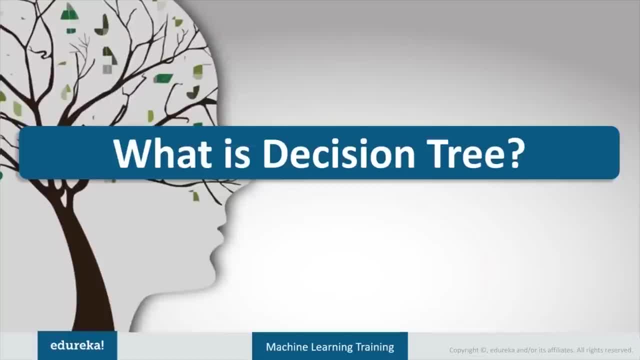 a given data set, you cannot say that the classifier has made that particular decision tree. it's like you cannot say that this algorithm performs better than that. it's like you cannot say that decision tree is better than name bias or name bias is performing better than decision tree. 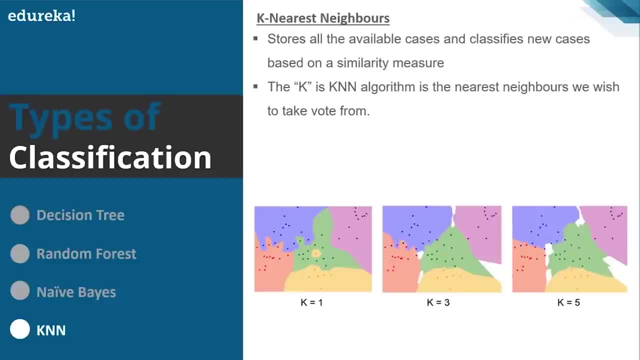 are using the register are in fact stealing customers personal information, or if a register data indicates that a particular good is being returned or exchanged multiple times, This could indicate that employees are misusing the return policy or trying to make money from doing the fake returns. 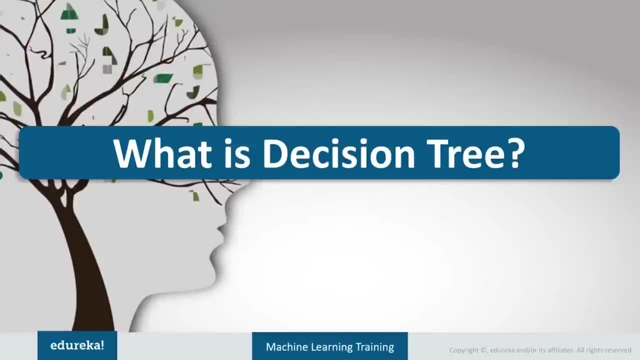 right, So this was about KNN algorithm. So, starting with, what is decision tree? but first let me tell you why do we choose decision tree to start with. Well, these decision tree are really very easy to read and understand. It belongs to one of the few models that are interpretable. 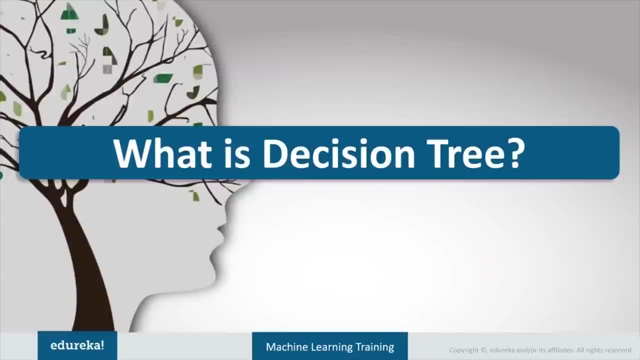 where you can understand exactly why the classifier has made that particular decision Right. Let me tell you a fact: that, for a given data set, you cannot say that this algorithm performs better than that. It's like you cannot say that decision trees better than neighbor. 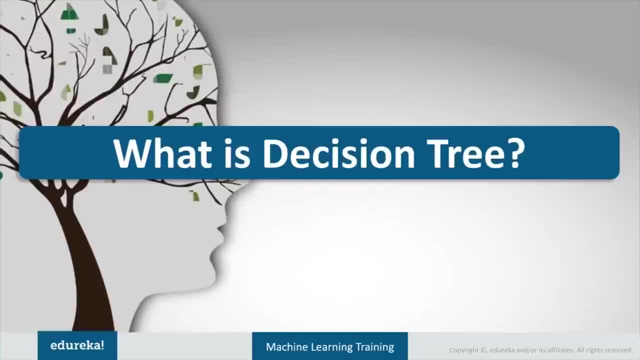 is or neighbor, is performing better than decision tree. It depends on the data set right. You have to apply hidden trial method with all the algorithm One by one and then compare the result. the model which gives the best result is the model which you can use it for better. 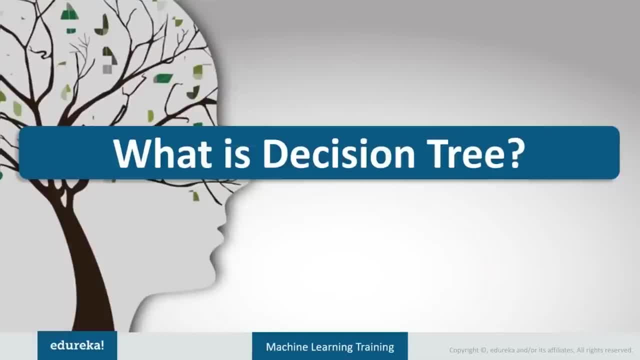 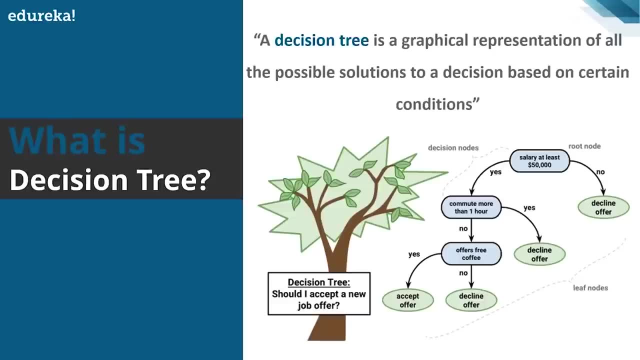 accuracy for your data set. All right, So let's start with. what is decision tree? Well, a decision tree is a graphical representation of all the possible solution to a decision based on certain conditions. Now you might be wondering why this thing is called as. 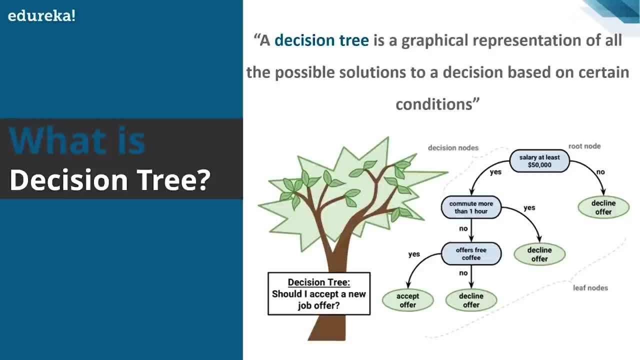 decision tree. Well, it is called so because it starts with a root and then branches off to a number of solution, Just like a tree, right? Even the tree starts from a root and it starts growing its branches Once it gets bigger and bigger. 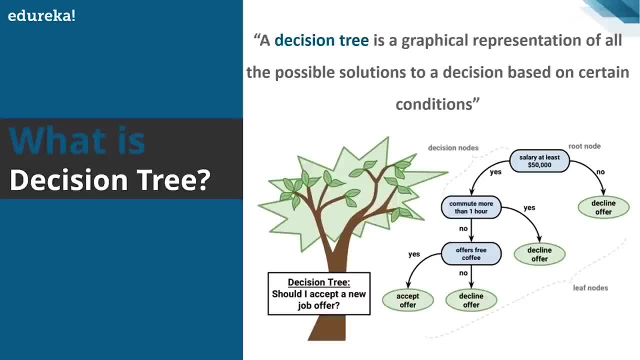 Similarly in a decision tree. It has a rule which keeps on growing with increasing number of decision and the conditions. Now let me tell you a real life scenario. I won't say that all of you, but most of you, must have used it. 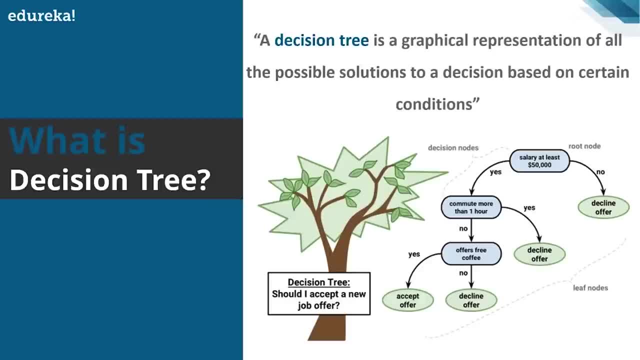 Remember, whenever you dial the toll-free number of your credit card company, it redirects you to his intelligent computerized assistant where it asks you questions like press 1 for English or press 2 for Hindi, Press 3 for this, press 4 for that. right now. 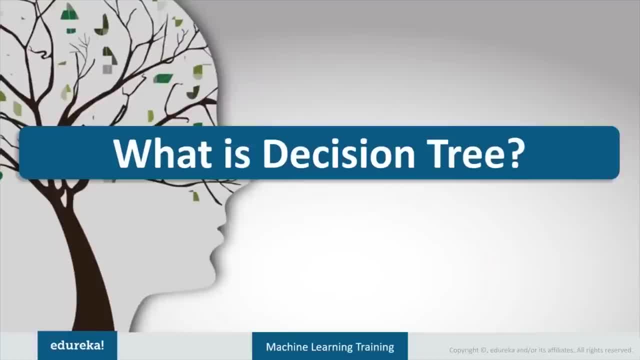 it depends on the data set, right? you have to apply hidden trial method with all the algorithms one by one and then compare the result. the model which gives the best result is the model which you can use it for better accuracy for your data set. all right, so let's start with what is decision tree? 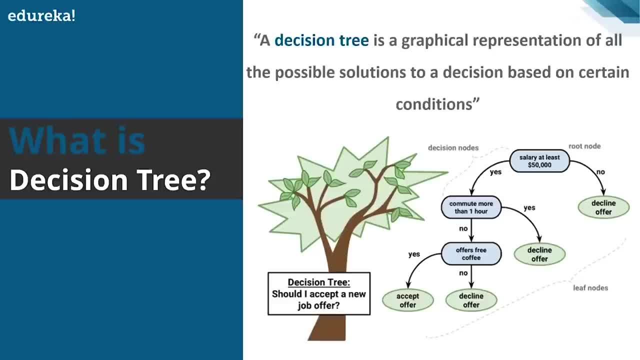 well, a decision tree is a graphical representation of all the possible solution to a decision based on certain conditions. now you might be wondering why this thing is called as decision tree. well, it is called so because it starts with a root and then branches off to a number of solution, just like a tree, right even. the tree starts from a root and it starts growing its 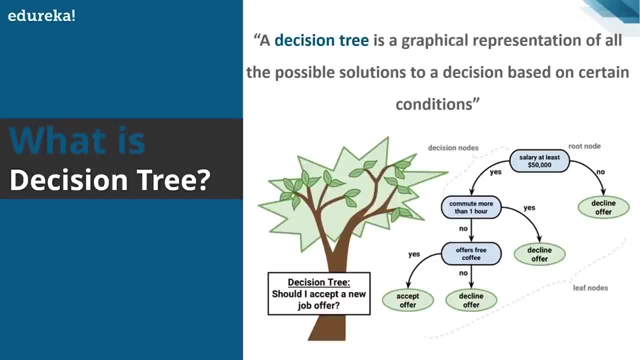 branches once it gets bigger and bigger. similarly, in a decision tree, it has a root which keeps on growing with increasing number of decision and the conditions. now let me tell you a real life scenario. let's say that all of you, but most of you, must have used it. remember whenever you dial the toll. 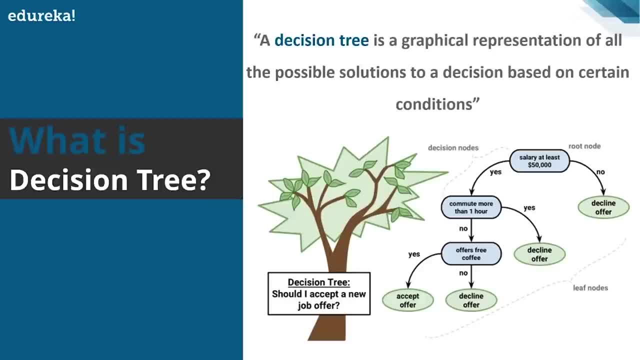 free number of your credit card company. it redirects you to his intelligent computerized assistant where it asks you questions like press 1 for english or press 2 for hindi, press 3 for this, press 4 for that right now. once you select one, now again it redirects you to a certain set of 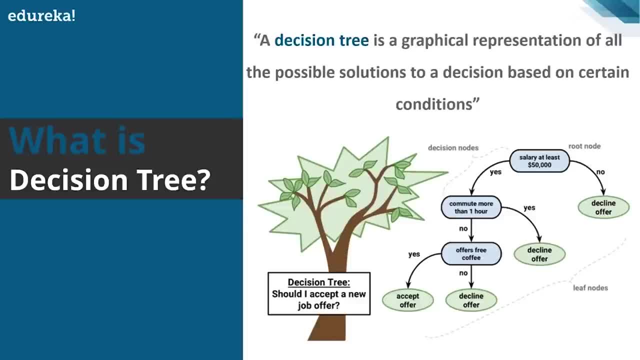 questions like press 1 for this, press 1 for that and similarly right. so this keeps on repeating until you finally get to the right person. right, you are caught in a voicemail hell. but what the company was actually doing, it was just using a decision tree to get you to the right person. all right, i'd like you to focus on this particular 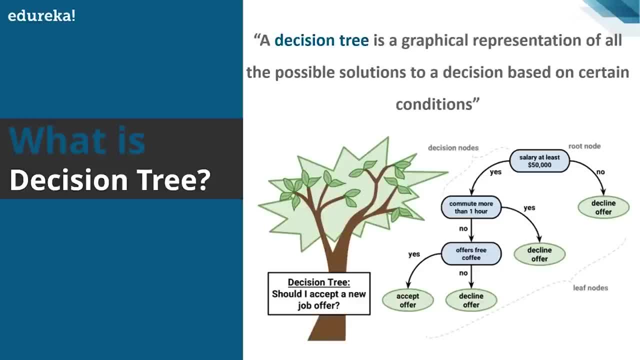 image for a moment. on this particular slide you can see image where the task is. should i accept a new job offer or not? all right, so you have to decide that. for that what you did, you created a decision tree starting with the base condition or the root node. was that the basic salary or 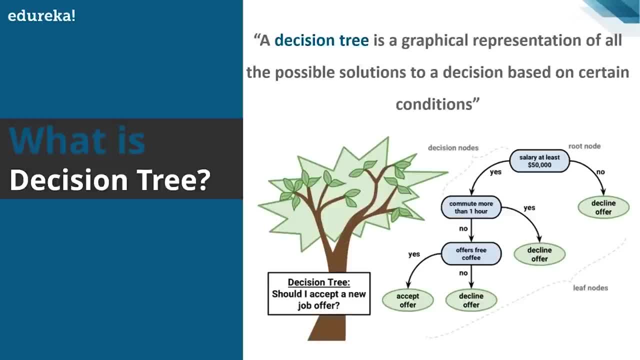 the minimum salary should be fifty thousand dollars. if it is not fifty thousand dollars, then you are not at all accepting the offer. all right, so if your salary is greater than fifty thousand dollar, then you will further check whether the commute is more than one hour or not. 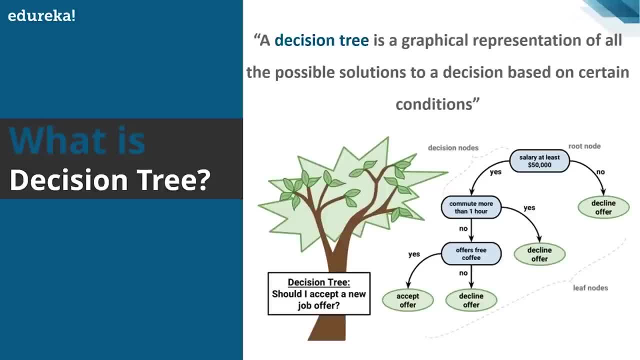 Once you select one, now again it redirects you to a certain set of questions like press 1 for this, press 1 for that and similarly right. So this keeps on repeating until you finally get to the right person, right? You might think that you are caught in a voicemail- hell, but 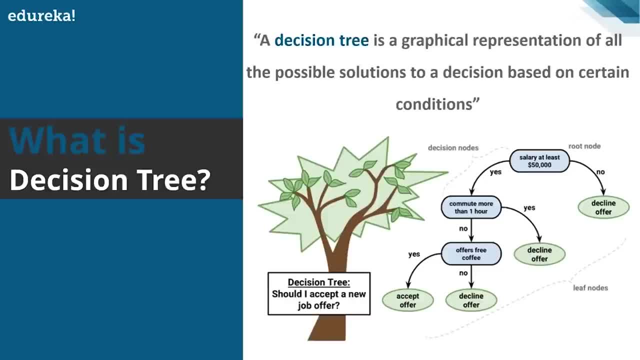 what the company was actually doing. it was just using a decision tree to get you to the right person allied. I'd like you to focus on this particular image for a moment. on this particular slide, You can see image where the task is: Should I accept a new job offer or not? 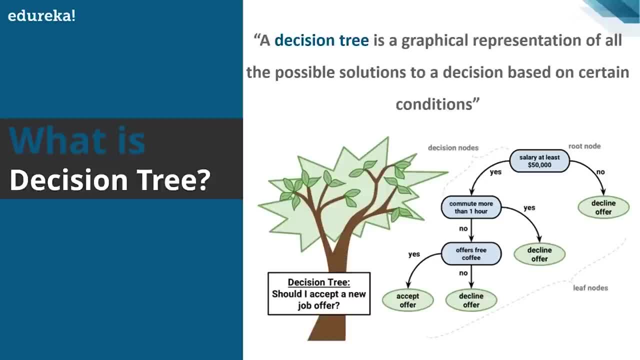 All right, so you have to decide that. but that what you did- you created a decision tree starting with the base condition, or the root node- was that the basic salary, or the minimum salary, should be $50,000.. If it is not $50,000, then you are not at all accepting the offer a late. So if your salary is greater than $50,000, then you will further check whether the commute is more than one hour or not. If it is more than one hour, you will just decline the offer. if it is less than one hour, then you are getting closer. 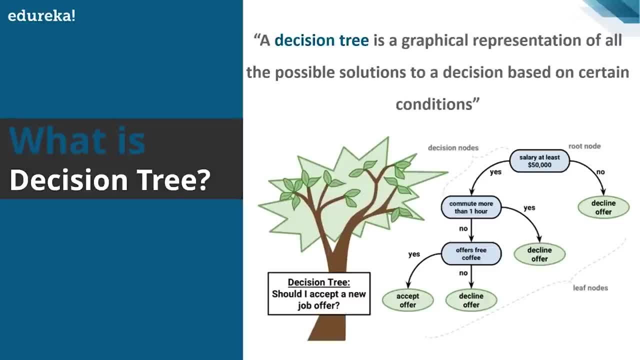 to accepting the job offer. Then, further what you'll do, you will check whether the company is offering free coffee or not. right, If the company is not offering the free coffee, then you will just decline the offer and have fitters offering the free. 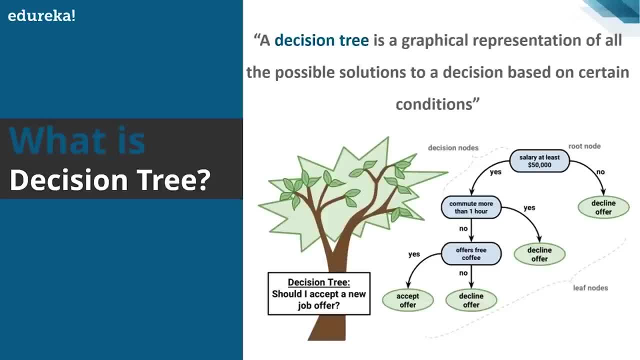 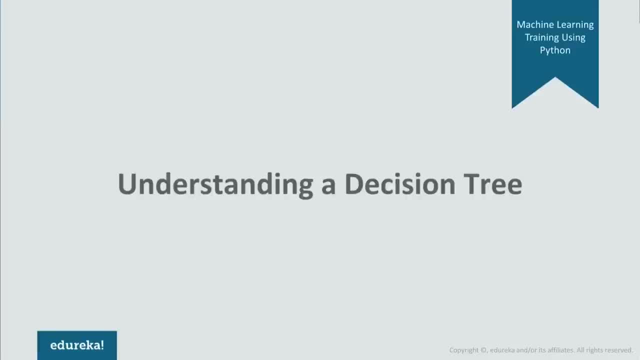 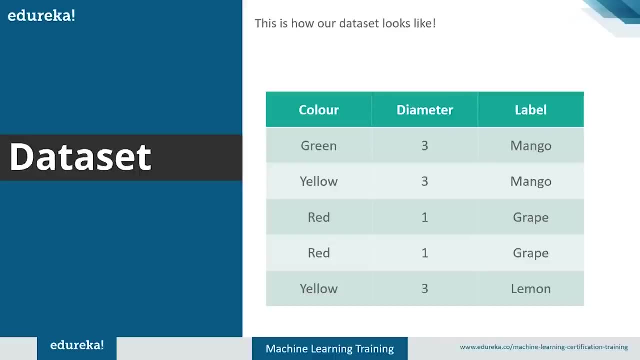 coffee and yeah, you will happily accept the offer, right? These are just our example of a decision tree. Now let's move ahead and understand a decision tree. Well, here is a sample data set that I'll be using it to explain. 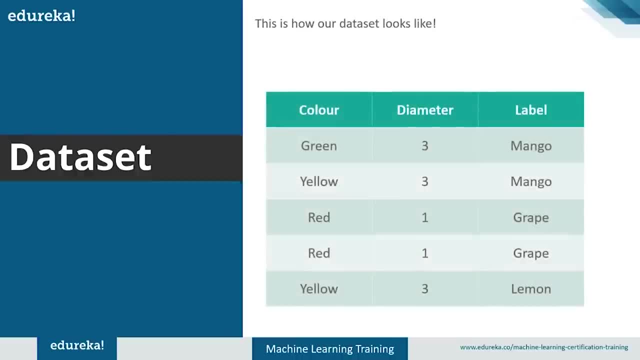 you about the decision tree. All right, in this data set, each row is an example and the first two columns provide features or attributes. that describes the data and the last column gives the label or the class we want to predict. and, if you like, you can just modify this data by. 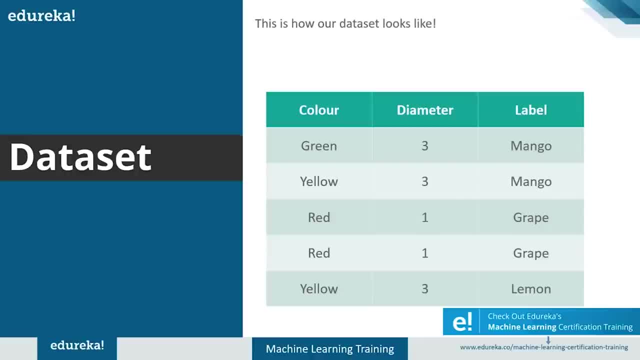 adding additional features and more example, and our program will work in exactly the same way. fine, Now, this data set is pretty straightforward, except for one thing. I hope you have noticed that it is not perfectly separable. Let me tell you Something more about that, as in the second and fifth examples, 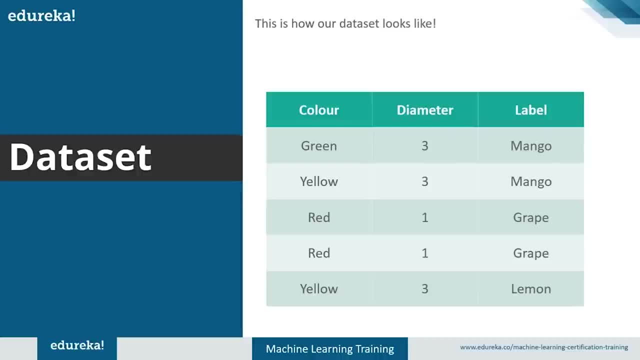 they have the same features but different labels. both have yellow as their color and diameter as three, but the labels are mango and lemon. fine, Let's move on and see how our decision tree handles this case. All right, in order to build a tree, will use a decision tree. 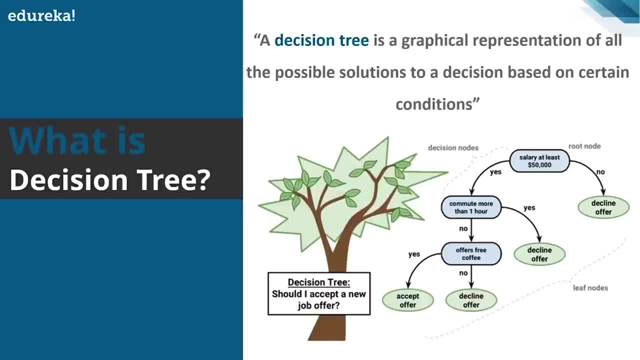 if it is more than one hour, you will just decline the offer. if it is less than one hour, then you are getting closer to accepting the job offer. then, further, what you'll do, you will check whether the company is offering free coffee or not. right, if the company is not offering the free coffee, then 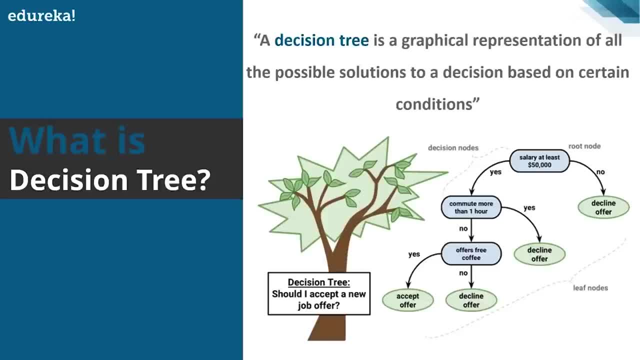 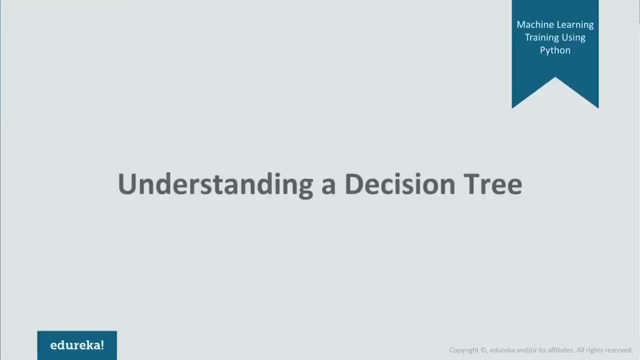 you will just decline the offer. and if it is offering the free coffee, then yeah, you will happily accept the offer. right? These are just our example of a decision tree. Now let's move ahead and understand a decision tree. Well, here is a sample data set that I'll be using it. 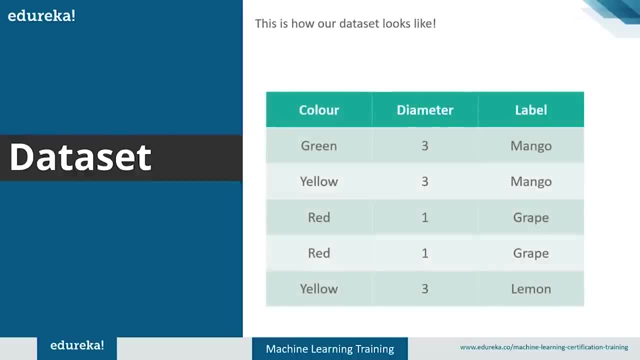 to explain you about the decision tree. All right, in this data set, each row is an example and the first two columns provide features or attributes. that describes the data and the last column gives the label or the class we want to predict and, if you like, you can just modify this data. 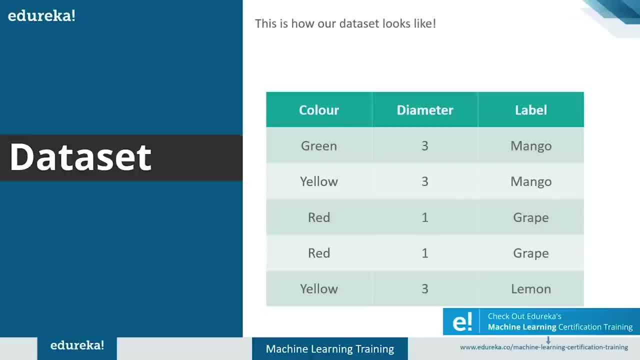 by adding additional features and more example, and our program will work in exactly the same way. fine, Now, this data set is pretty straightforward, except for one thing. I hope you have noticed that it is not perfectly separable. Let me tell you something more about that. as in the second, 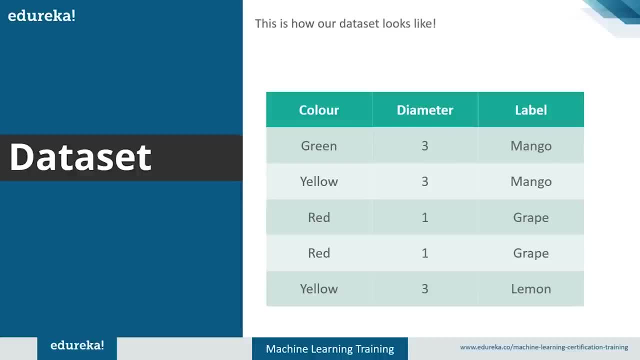 and fifth examples. They have the same features but different labels. both have yellow as their color and diameter as three, but the labels are mango and lemon. fine, Let's move on and see how our decision tree handles this case. All right, in order to build a tree. 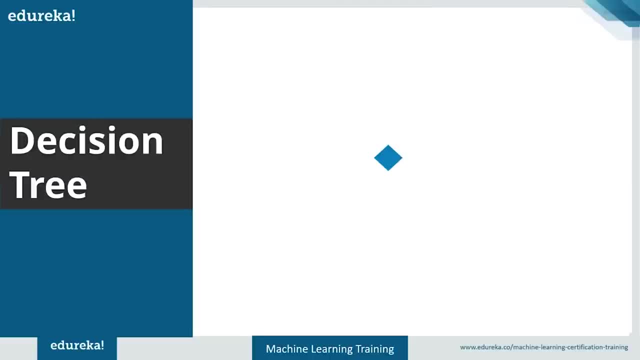 We'll use a decision tree algorithm called card. The Scott algorithm stands for classification and regression tree algorithm. All right, Let's see a preview of how it works. All right, to begin with, we'll add a root node for the tree and all the nodes receive a list of rows as input. 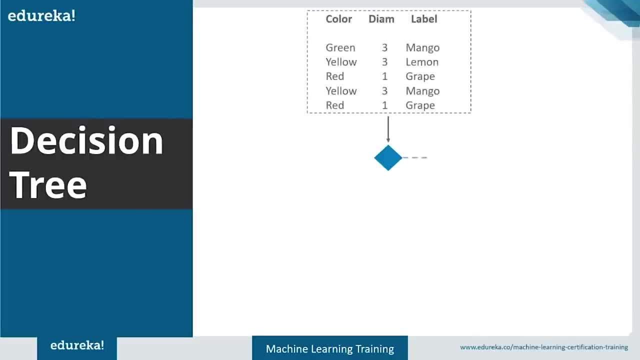 and the route will receive the entire training data set. Now each node will ask- true and false- question about one of the feature and in response to that question We will split or partition the data set into two different subsets. These subsets then become input to two child node. 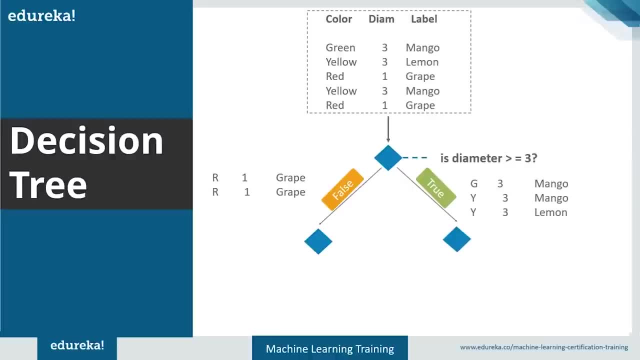 We add to the tree, and the goal of the question is to finally unmix the labels as we proceed down, or in other words, to produce the purest possible distribution of the labels at each node. For example, the input of this node contains only one single type of label. 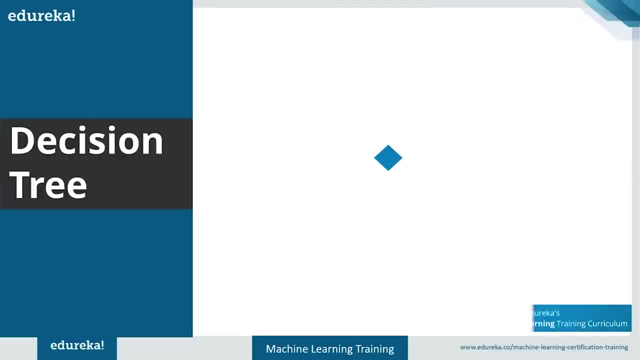 algorithm called cart. The Scott algorithm stands for classification and regression tree algorithm. All right, let's see a preview of how it works. All right, To begin with will add a root node for the tree and all the nodes receive a list of rows as input and the route will receive 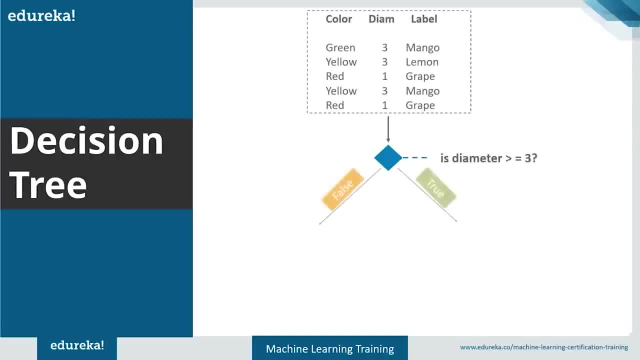 the entire training data set. Now each node will ask- true and false- question about one of the feature and in response to that question, will split or partition the data set into two different subsets. these subsets then become input to child node. We are to the tree and the goal of the question is to finally 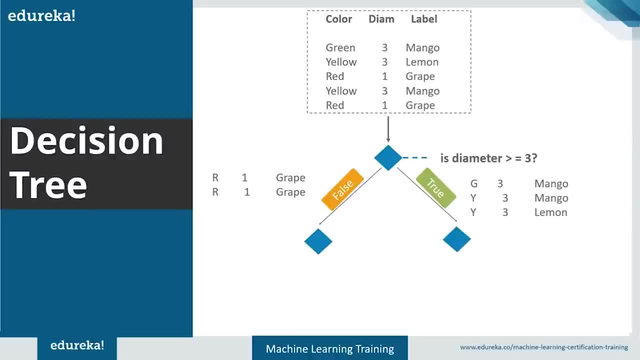 unmix the labels as we proceed down, or in other words, to produce the purest possible distribution Of the labels at each node. For example, the input of this node contains only one single type of label, so we could say that it's perfectly unmixed. 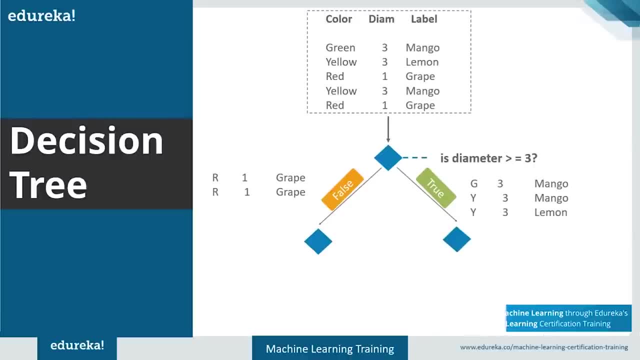 There is no uncertainty about the type of label, as it consists of only grapes right. on the other hand, the labels in this node are still mixed up, So we would ask another question to further drill it down. right, but before that we need to understand which question to ask. 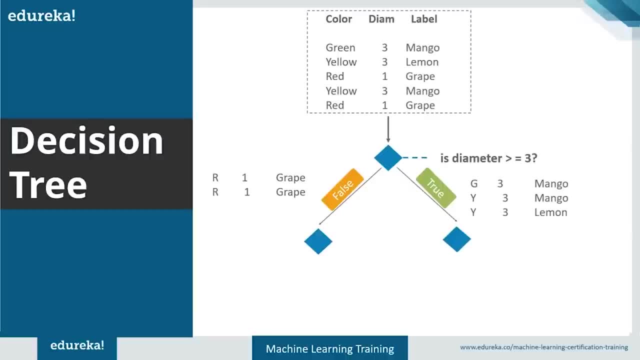 and when. and to do that We need to quantify how much question helps to unmix the label. and we can quantify the amount of uncertainty at a single node using a metric called Jenny impurity. and we can quantify how much a question reduces that uncertainty using 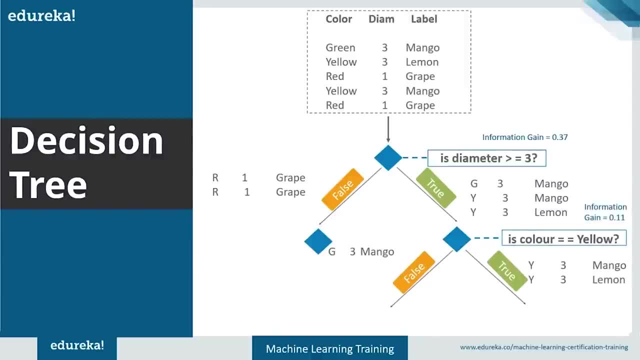 a concept called information game, will use these to select the best question to ask at each point, and then what we'll do will iterate. the steps will recursively build the tree on each of the new node, will continue dividing the data until there are no further question to ask and finally we reach to. 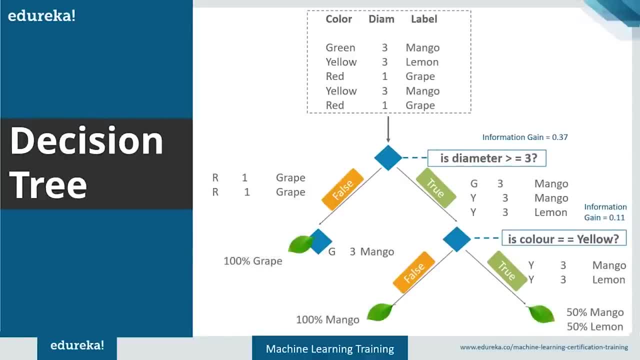 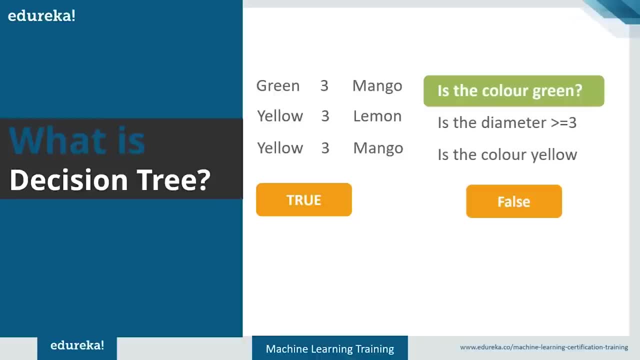 our leave, All right, all right, So this was about decision tree. So, in order to create a decision tree, first of all, what do you have to do? You have to identify different set of questions that you can ask to a tree, like: is this color green and what will be these? 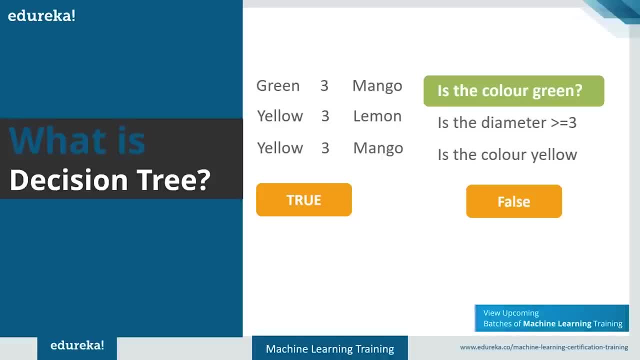 question. these questions will be decided by your data set like: is this color green? is the diameter greater than equal to three? is the color yellow? right questions resembles to your data set. Remember that, All right, So if my color is green, then what it will do? it will divide. 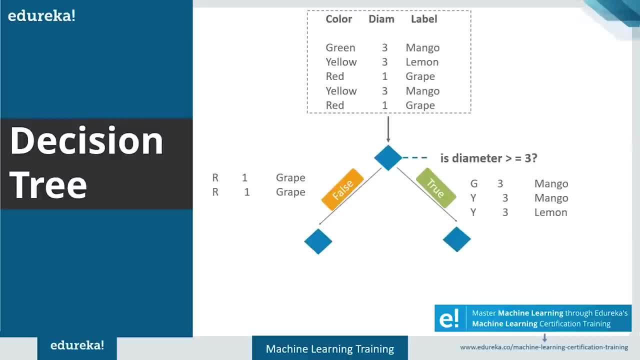 So we could say that it's perfectly unmixed. There is no uncertainty about the type of label, as it consists of only grapes Right. on the other hand, the labels in this node are still mixed up, So we would ask another question to further drill it down, right. 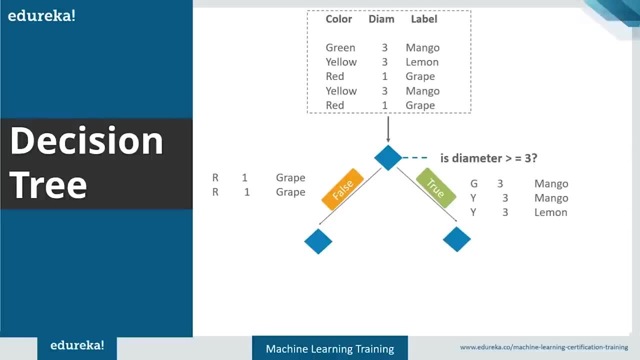 But before that we need to understand which question to ask and when. and to do that, we need to quantify how much question helps to unmix the label, and we can quantify the amount of uncertainty at a single node using a metric called Ginny impurity, and we can quantify how much a question reduces. 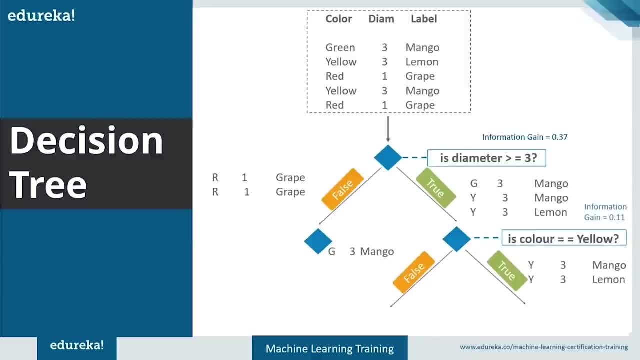 that uncertainty. using a concept called information game, We'll use these to select the best question to ask at each point, and then what we'll do will iterate. the steps will recursively build the tree on each of the new node, will continue dividing the data until there are no further question to ask. 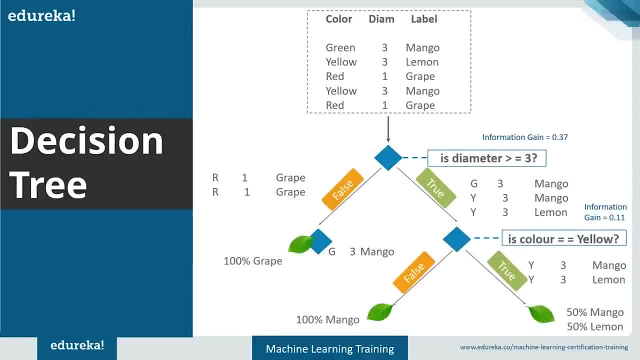 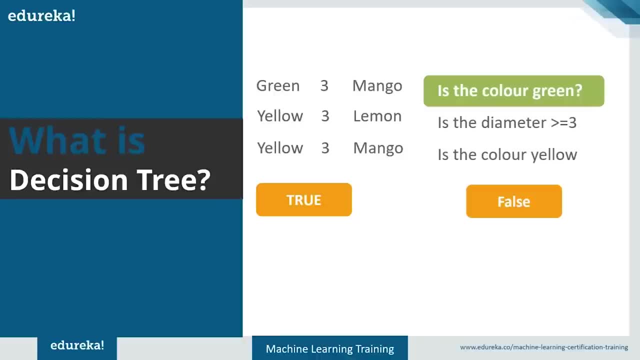 and finally we reach to our leaf. All right, All right. So this was about decision tree. So, in order to create a decision tree, first of all, what do you have to do? You have to identify different set of questions that you can ask to a tree, like: is this color green? 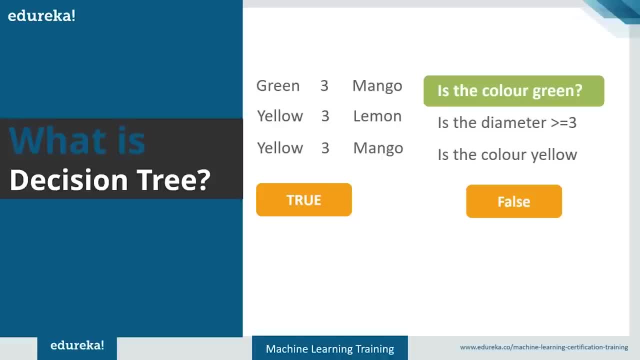 and what will be these question? these question will be decided by your data set, like: is this color green as the diameter greater than or equal to 3? is the color yellow right questions resembles to your data set. Remember that. all right. So if my color is green, 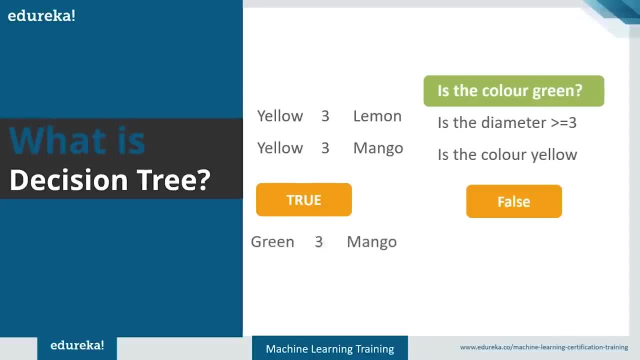 then what it will do. it will divide into two parts. first, The green mango will be in the true, while on the false We have lemon and the mango. All right if the color is green, or the diameter is greater than or equal to 3, or the color is yellow. 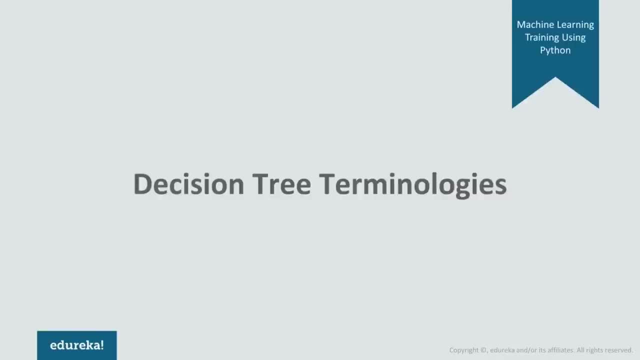 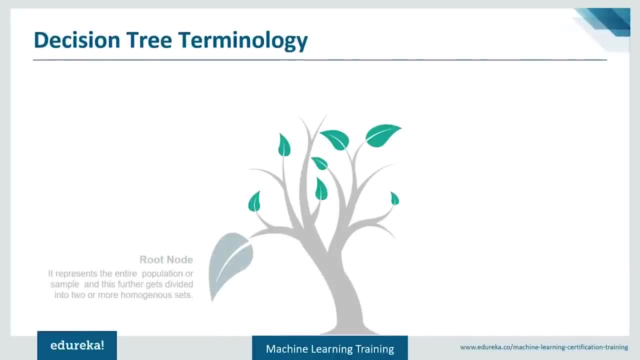 Now let's move on and understand about decision tree terminologies. All right, so starting with root node, root node is the base node of a tree. the entire tree starts from a root node. In other words, It is the first node of a tree, it represents the entire. 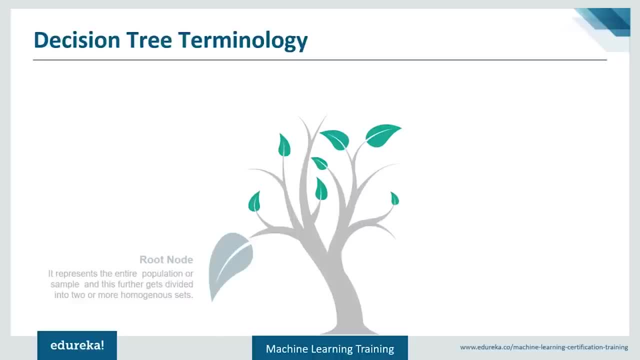 population or sample, and this entire population is further segregated or divided into two or more homogeneous set fine. Next is the leaf node. Well, leaf node is the one when you reach at the end of the tree, right that is. you cannot further segregated down to any. 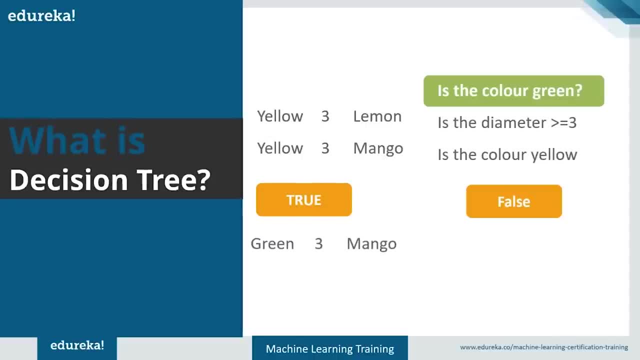 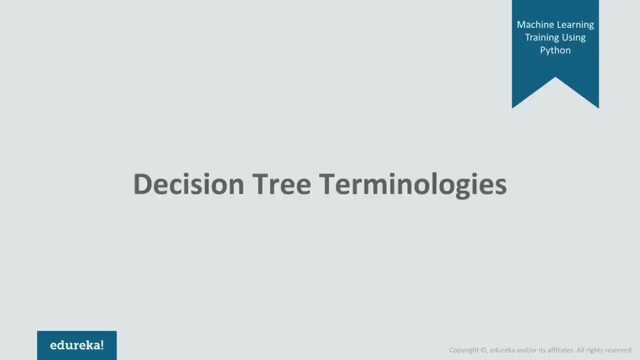 into two parts. First, the green mango will be in the true, while on the false we have lemon and the mango. all right, if the color is green, or the diameter is greater than equal to three, or the color is yellow. Now let's move on and understand about decision tree terminologies. 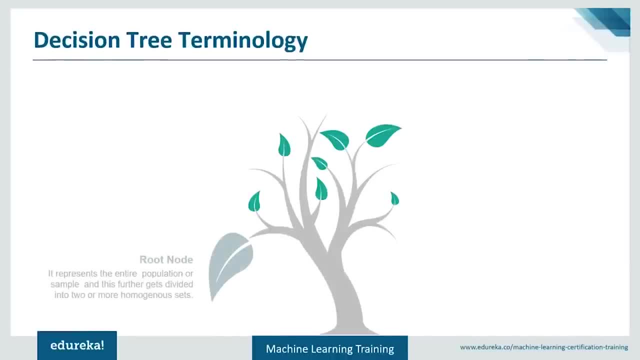 all right. So, starting with root node, root node is the base node of a tree. The entire tree starts from a root node. In other words, it is the first node of a tree. It represents the entire population or sample, and this entire population is further segregated or divided into two or more. 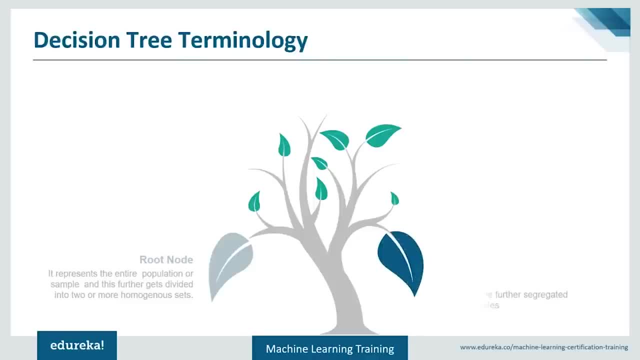 homogeneous set fine. Next is the leaf node. Well, leaf node is the one when you reach at the end of the tree, right that is. you cannot further segregated down to any other level. that is the leaf node. next is splitting. splitting is dividing your root node or your node into different sub. 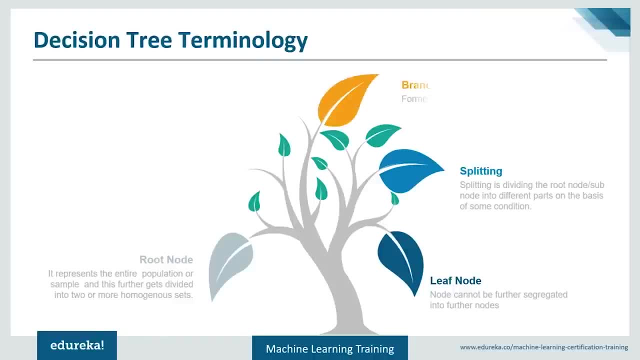 part on the basis of some condition. All right. then comes the branch or the sub tree. Well, this branch or sub tree gets formed when you split the tree. suppose, when you split a root node, it gets divided into two branches or two sub trees. right next is the concept of 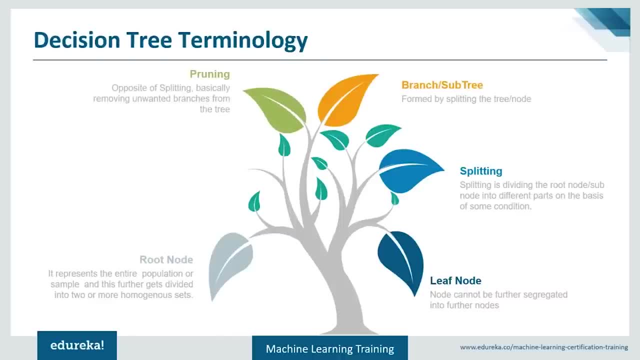 pruning. Well, you can say that pruning is just opposite of splitting. what we are doing here. We are just removing the sub node of a decision tree. We'll see more about pruning later in this session. All right, let's move on ahead. next is parent or child node. 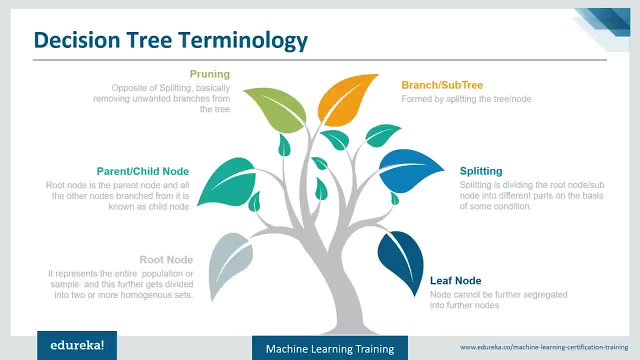 Well, First of all, Root node is always the parent node and all other nodes associated with that is known as child node. Well, you can understand it in a way that all the top node belongs to a parent node and all the bottom node, which are 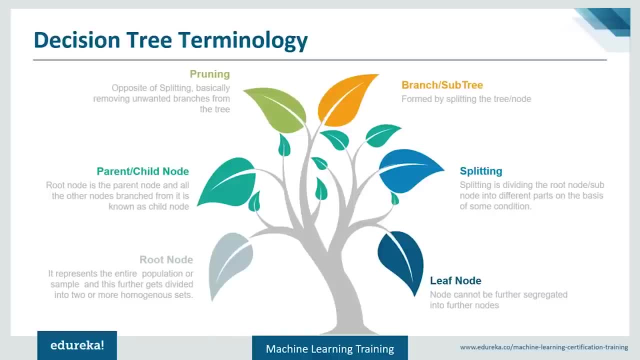 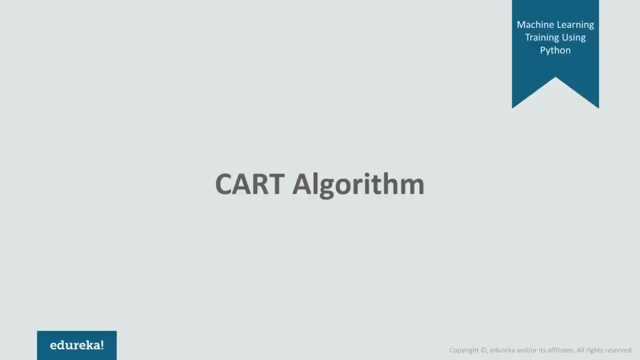 derived from a top node is a child node. The node producing a further node is a child node and the node which is producing it is a parent node. simple concept, right? Let's use the cart algorithm and design In a tree manually. So, first of all, what do you do? you decide which question to. 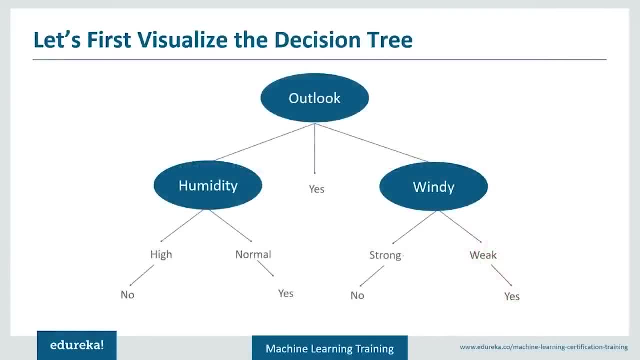 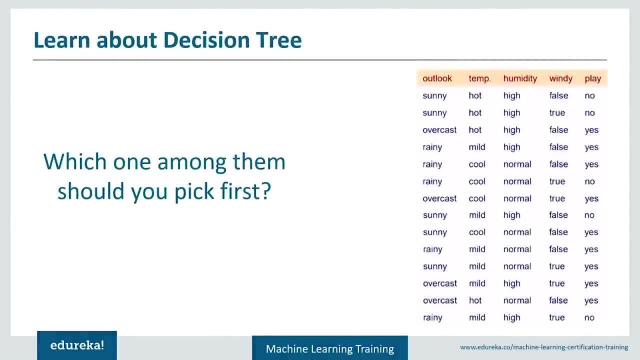 ask and when? so how will you do that? So let's first of all visualize the decision tree. So there's the decision tree which will be creating manually on like. first of all, let's have a look at the data set. You have Outlook, temperature, humidity and windy as your. 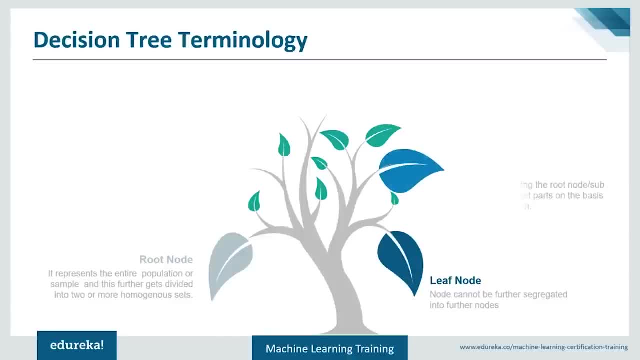 other level, that is the leaf node. next is splitting. splitting is dividing your root node or your node into different sub part on the basis of some condition. All right, then comes the branch or the subtree. Well, this branch or subtree gets formed when you split the 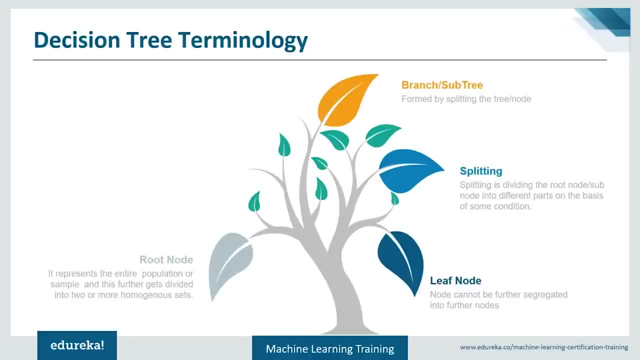 tree. suppose, when you split a root node, it gets divided into two branches or two sub trees. right next is the concept of pruning. Well, you can say that Pruning is just opposite of splitting. what we are doing here. We are just removing the sub node of a decision tree. 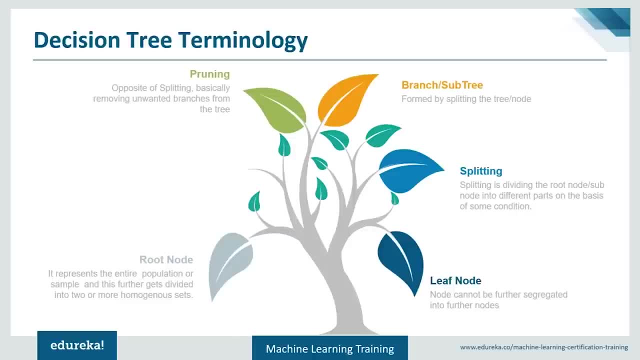 We'll see more about pruning later in this session. All right, let's move on ahead. next is parent or child node? Well, first of all, root node is always the parent node, and all other nodes associated with that is known as child node. 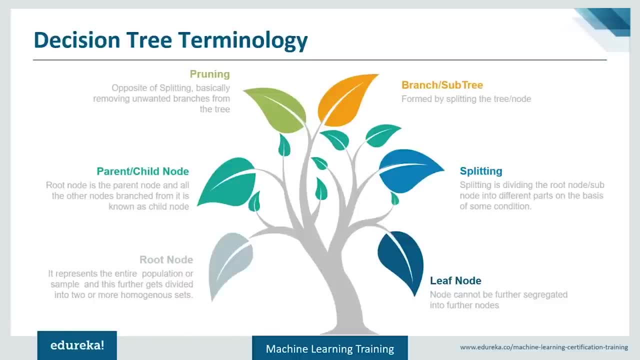 Well, you can understand it in a way that all the top node belongs to a parent node and all the bottom node which are derived from a top node is a child node. The node producing a further node is a child node and the node which is producing it is a parent node. simple concept. 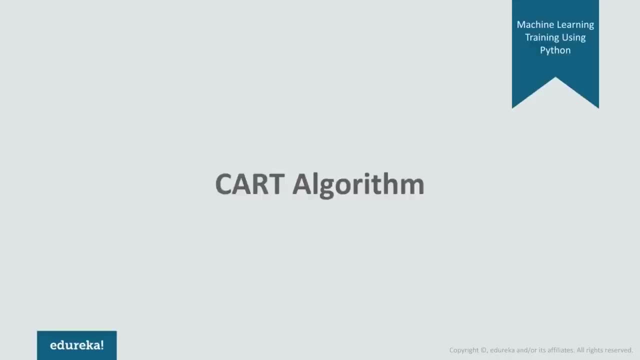 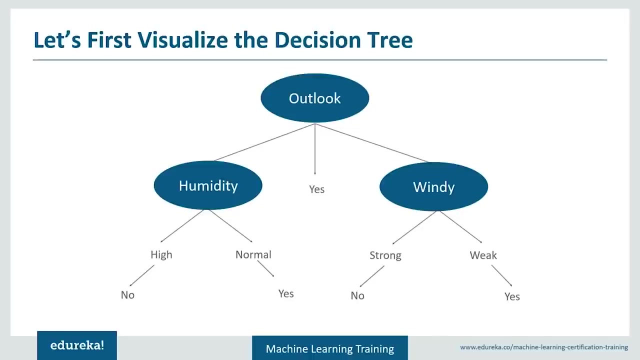 right, Let's use the cart algorithm and design a tree manually. So, first of all, what do you do? you decide which question to ask and when. so how will you do that? So let's first of all visualize the decision tree. So there's the decision tree which will be creating manually. 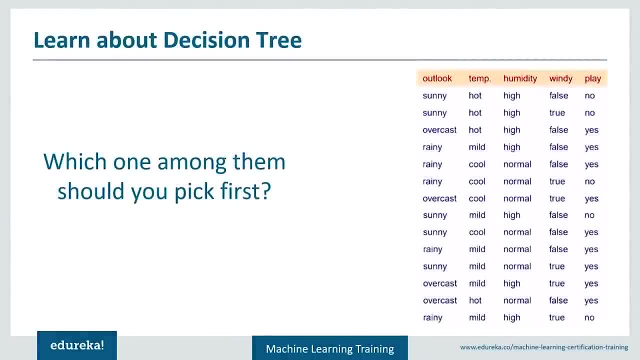 All right. First of all, let's have a look at the data set You have. Look temperature, humidity and windy as your different attribute. on the basis of that, you have to predict that, whether you can play or not. So which one among them should you pick first? answer determine. 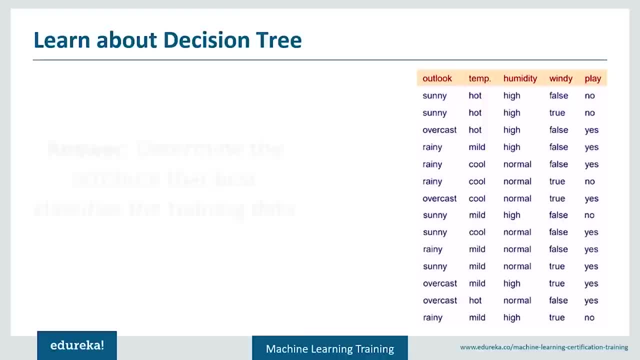 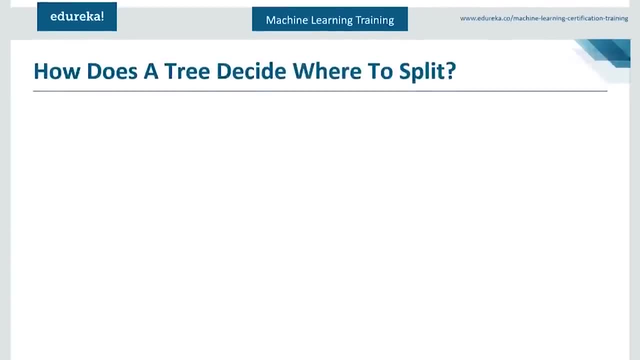 the best attribute that classifies the training data. All right, So how will you choose the best attribute? or how does a tree decide where to split? or how the tree will decide its root node? Well, before we move on and split a tree, There are some terminologies that you should know. 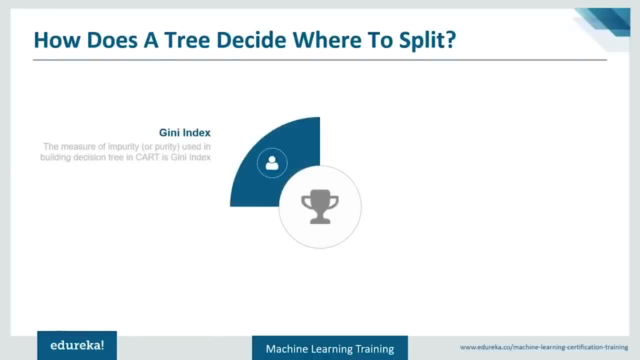 All right, first being the gene index. So what is this gene index? This gene index is the measure of impurity, of purity- used in building a decision tree in cart algorithm. All right. Next is information gain. This information gain is the decrease in entropy after data. 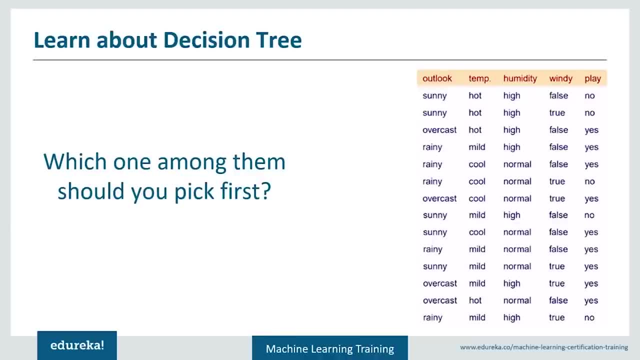 different attribute. on the basis of that, you have to predict that, whether you can play or not. So which one among them should you pick? first answer: determine the best attribute that classifies the training data. All right, So how will you choose the best attribute? or how does a tree? 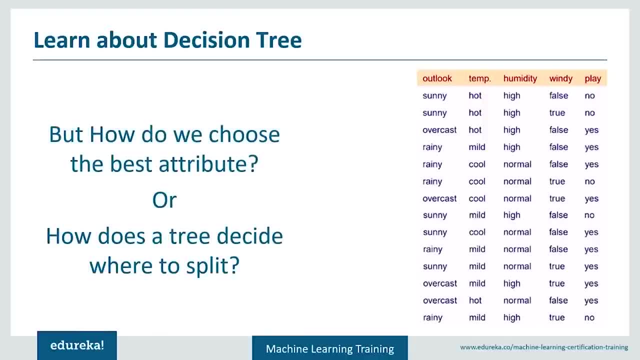 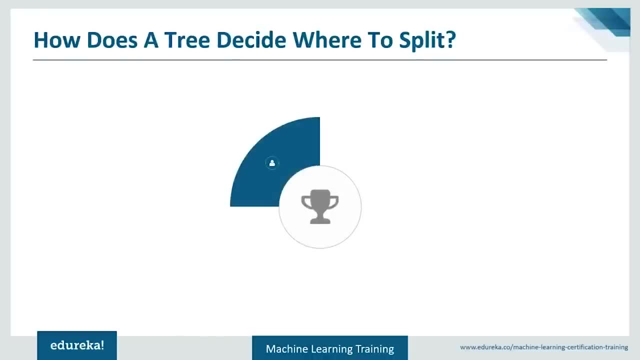 decide where to split or how the tree will decide its root node. Well, before we move on and split a tree, There are some terminologies that you should know All right, first being the gene index. So what is this gene index? This gene index is the measure of impurity, of purity, used in 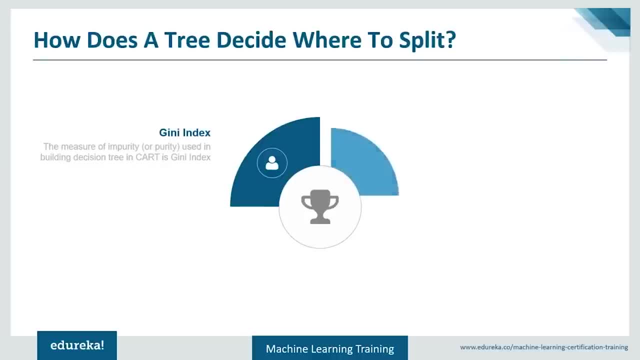 building a decision tree in cart algorithm: All right. Next is information gain. This information gain is the decrease in entropy after data set is split on The basis of an attribute. constructing a decision tree is all about finding a attribute that returns the highest information gain. 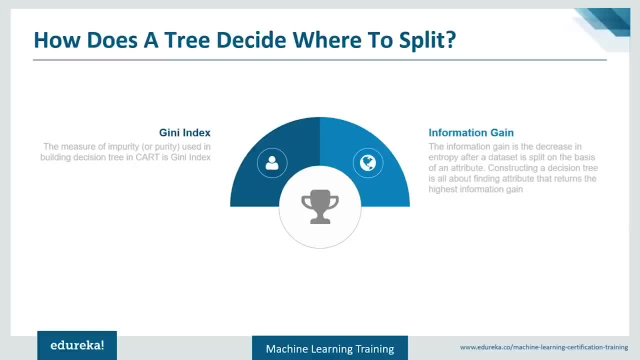 All right, so you'll be selecting the node that would give you the highest information gain. All right. Next is reduction in variance. This reduction in variance is an algorithm which is used for continuous target variable or regression problems. The split with lower variance is selected as a criteria to 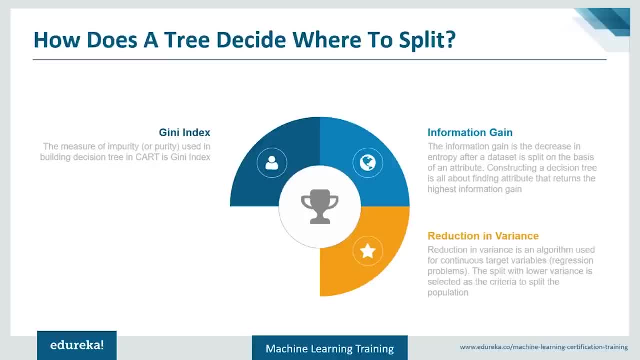 split the population. see in general term, What do you mean by variance? variance is how much your data is wearing right. So if your data is less impure or it is more pure than in that case, the variation would be less, as all the data are most. 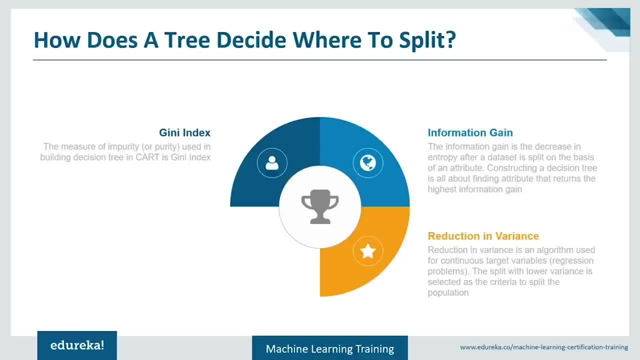 similar right. So there's also a way of splitting a tree. The split with lower variance is selected as a criteria to split the population. All right. Next is the chi-square. chi-square: It is an algorithm which is used to find out the statistical. 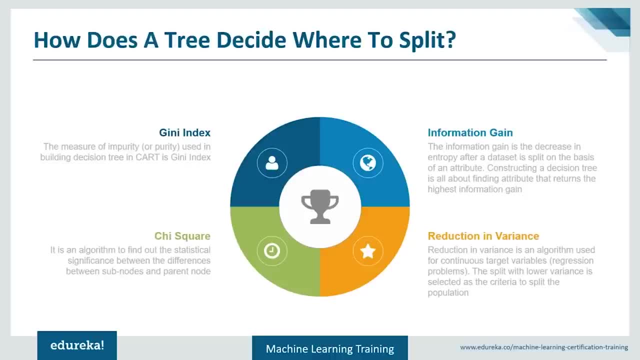 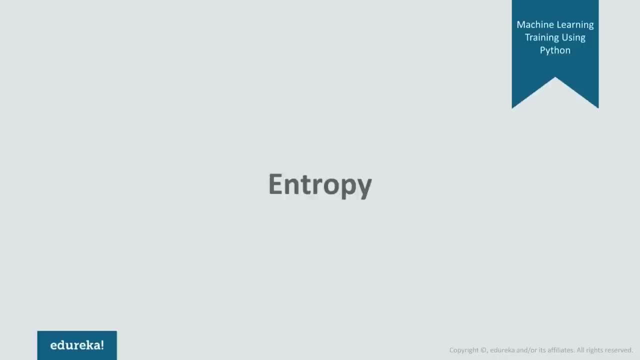 significance between the differences between sub nodes and the parent nodes. Fine, Let's move ahead Now. The main question is: how will you decide the best attribute for now? Just understand that you need to calculate something known as information gain. The attribute with the highest information gain is considered. 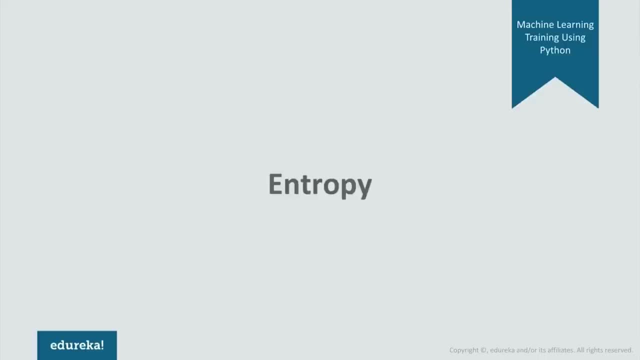 the best. Yeah, I know your next question might be like: what is this information again? but before we move on and see what exactly information gain is, let me first introduce you to a term called entropy, because this term will be used in calculating the information. 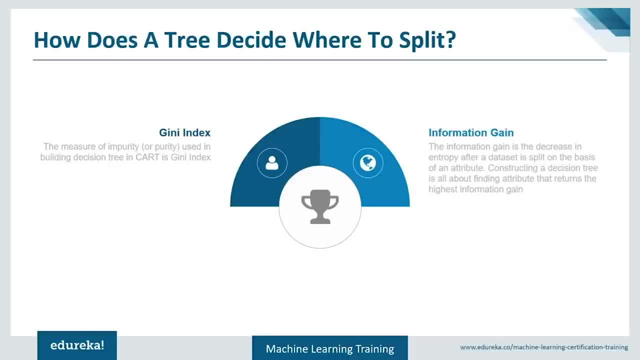 set is split on the basis of an attribute. constructing a decision tree is all about finding a attribute that returns the highest information gain. All right, so you'll be selecting the node that would give you the highest information gain, All right. Next is reduction in variance. this reduction in variance is: 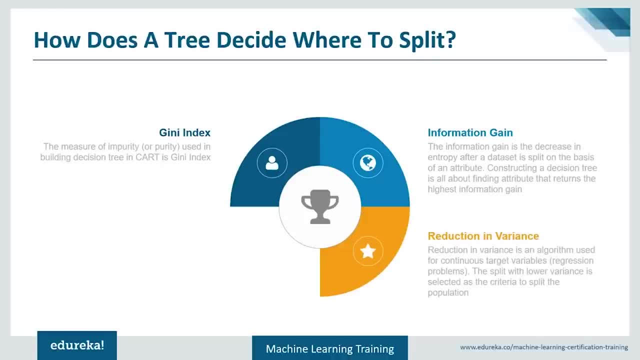 an algorithm which is used for continuous target variable or regression problems. The split with lower variance is selected as a criteria to split the population. see in general term. What do you mean by variance? Variance is how much your data is wearing right. So if your data is less impure or it is more pure than in 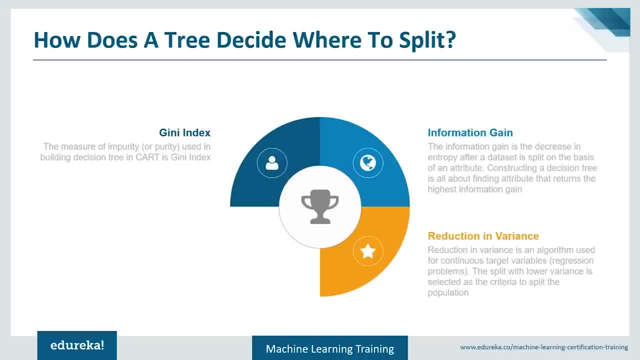 that case, the variation would be less, as all the data are more similar, right? So there's also a way of splitting a tree. the split with lower variance is selected as a criteria to split the population, All right. Next is the chi square. 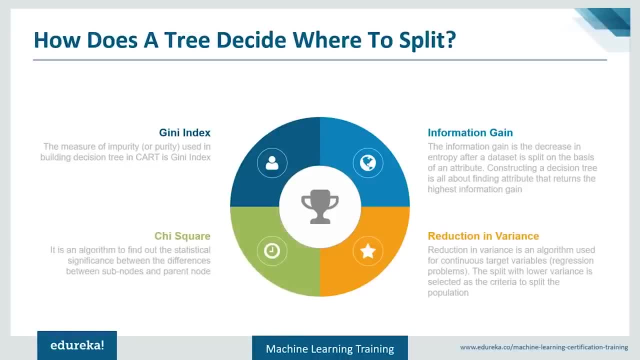 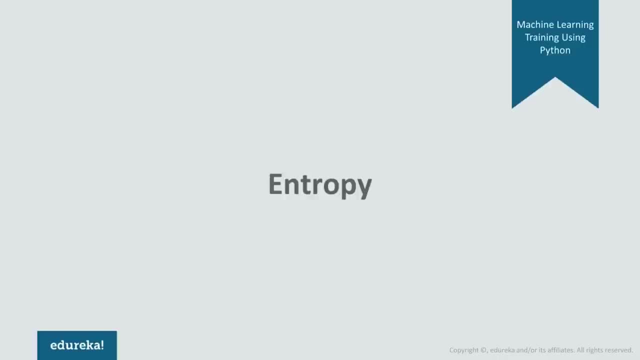 G square. It is an algorithm which is used to find out the statistical significance between the differences between sub nodes and the parent nodes. Fine, Let's move ahead Now. the main question is: how will you decide the best attribute for now? just understand that you need to calculate something. 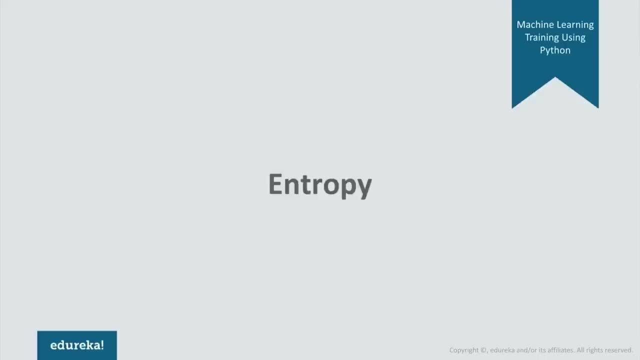 known as information gain. the attribute with the highest information gain is considered the best. Yeah, I know your next question might be like: what is this information gain? But before we move on and see what exactly information gain is, let me first introduce you to a term called entropy, because 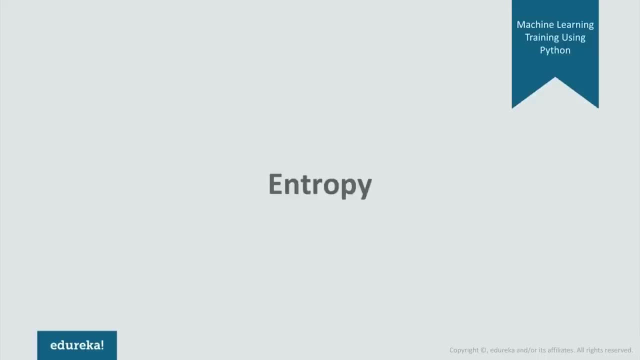 this term will be used in calculating the information gain will. entropy is just a metric which measures the impurity of something, or in other words, you can say that it's the first step to do before you solve the problem of a decision tree, as I mentioned here something about impurity. 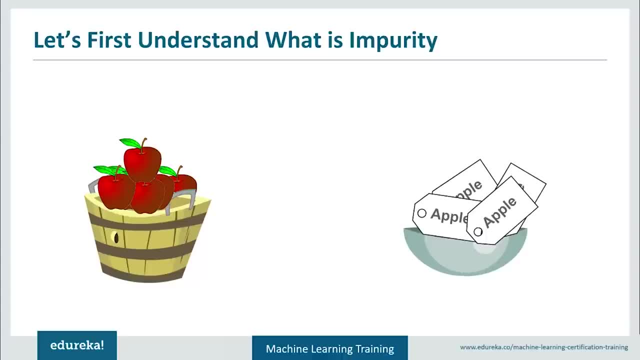 So let's move on and understand what is impurity. suppose you have a basket full of apples and another bowl which is full of same label, Which says Apple. now, if you are asked to pick one item from each basket and ball, then the probability of getting the apple 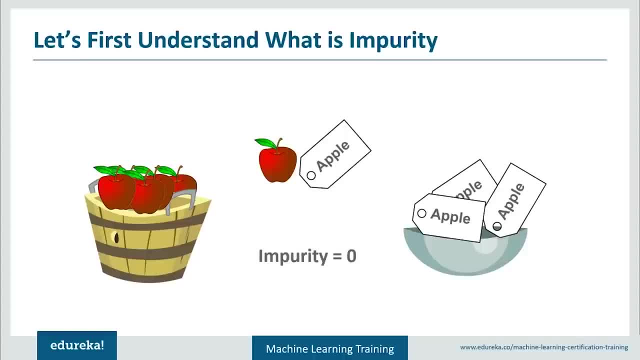 and its correct label is one. So in this case you can say that impurity is zero. All right, Now what if there are four different fruits in the basket and four different labels in the ball? then the probability of matching the fruit to a label is obviously not one. 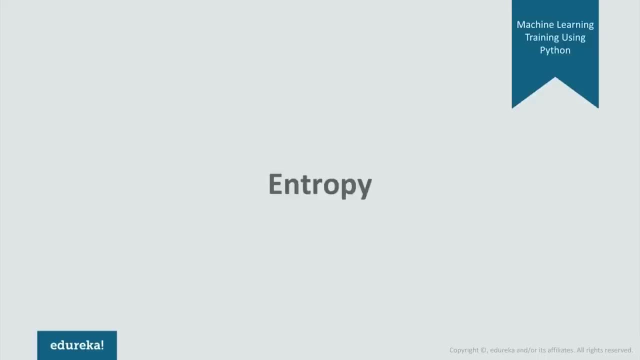 gain. Well, entropy is just a metric which measures the impurity of something, Or in other words, you can say that it's the first step to do before you solve the problem of a decision tree, as I mentioned here something about impurity. So let's move on and understand what is impurity, suppose you. 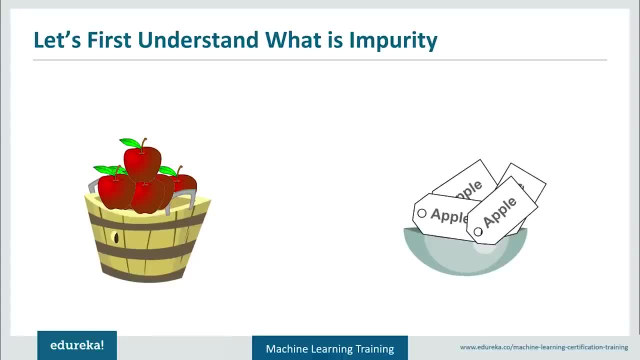 have a basket full of apples and another bowl which is full of same label, which says Apple. now, if you are asked to pick one item from each basket and ball, then the probability of getting the apple and its correct label is one. So in this case you can say that impurity is zero. 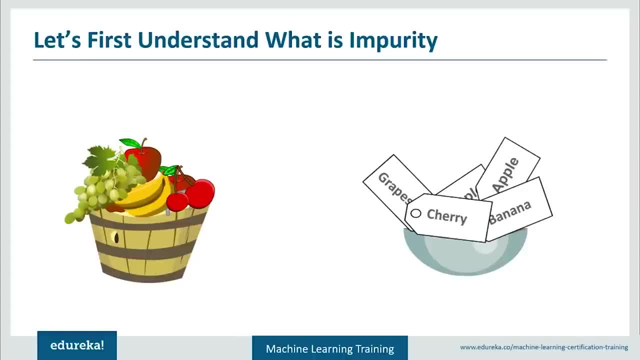 All right, Now What If there are four different fruits in the basket and four different labels in the ball? then the probability of matching the fruit to a label is obviously not one. It's something less than that. Well, it could be possible that I picked banana from the basket. 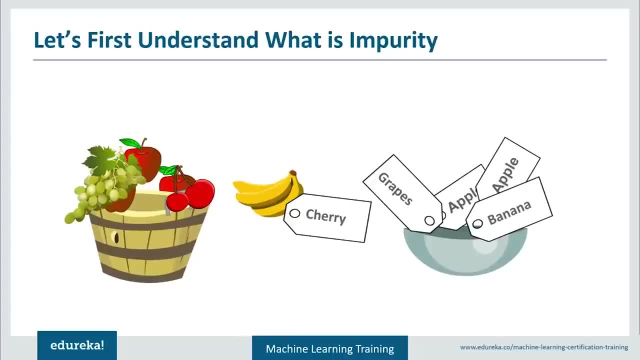 and when I randomly pick the label from the ball it says a cherry. any random permutation and combination can be possible. So in this case I would say that impurities is non-zero. I hope the concept of impurity is clear. So, coming back to entropy, as I said, entropy is. 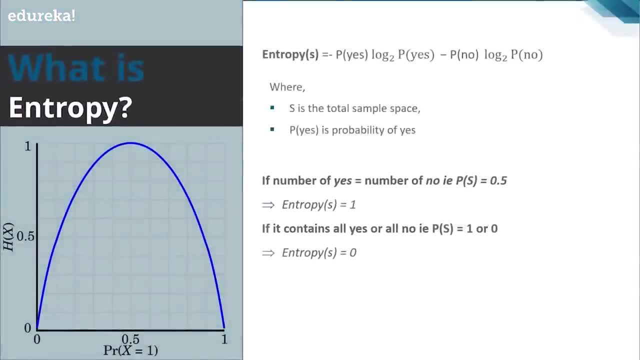 Measure of impurity. from the graph on your left You can see that as a probability is 0 or 1, that is, either they are highly impure or they are highly pure- then in that case the value of entropy is 0, and when the probability is, 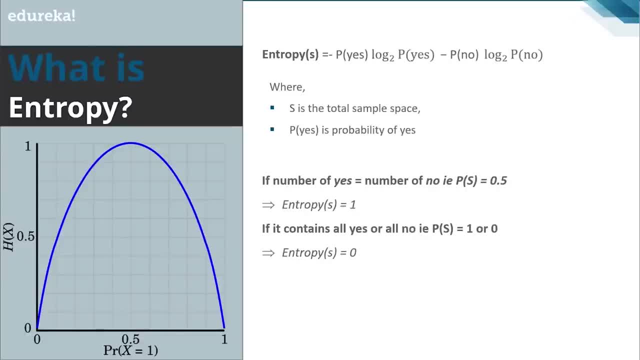 0.5, then the value of entropy is maximum. Well, what is impurity? impurity is the degree of randomness, how random a data is. so if the data is completely pure, in that case the randomness equals 0. or if the data is completely. 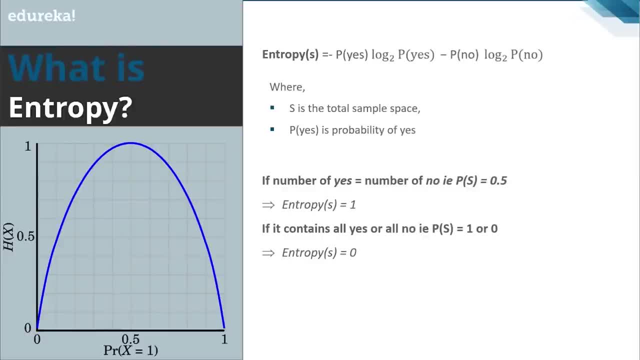 impure. even in that case, the value of impurity will be zero. Question like: why is it that the value of entropy is maximum at 0.5 might arise in your mind, right? So let me discuss about that. Let me derive it mathematically, as you can see here on the 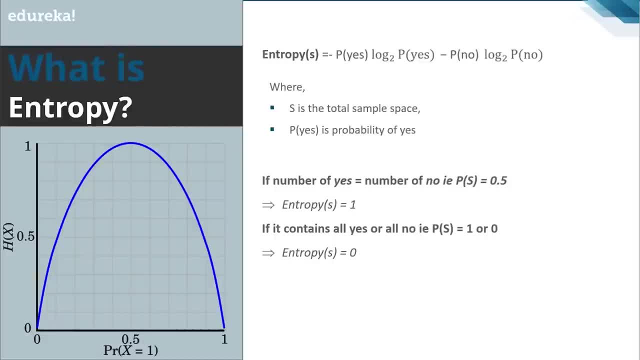 slide. the mathematical formula of entropy is minus of probability of yes. Let's move on and see what this graph has to say mathematically. suppose s is our total sample space and it's divided into two parts- Yes and no, like in our data set. the result for playing was: 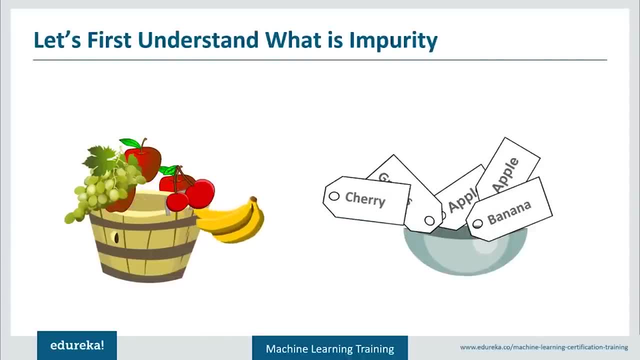 It's something less than that. Well, it could be possible that I picked banana from the basket and when I randomly pick the label from the ball, It says a cherry. any random permutation and combination can be possible, So in this case, I would say that impurities is nonzero. 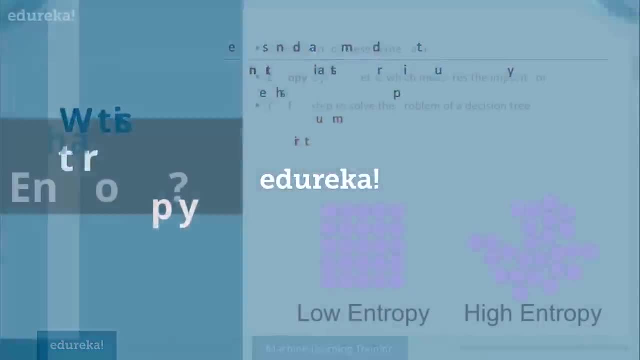 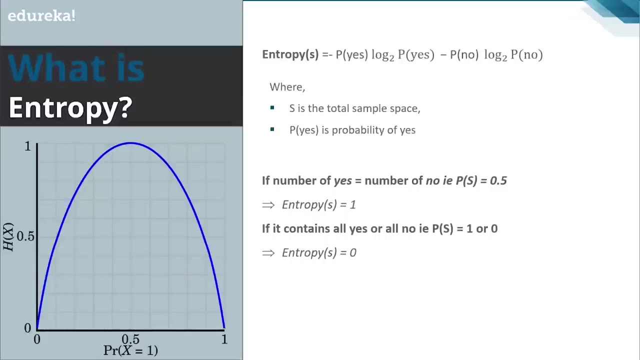 I hope the concept of impurity is clear. So, coming back to entropy, as I said, entropy is the measure of impurity. from the graph on your left You can see that, as the probability is 0 or 1, that is, either they are highly impure or they are highly pure, then in that, 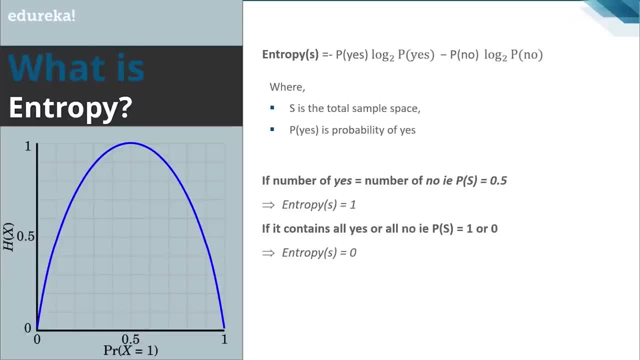 case the value of entropy is 0, and when the probability is 0.5, then the value of entropy is maximum. Well, what is impurity? impurity is the degree of randomness, how random a data is. So if the data is completely pure, in that case the randomness. 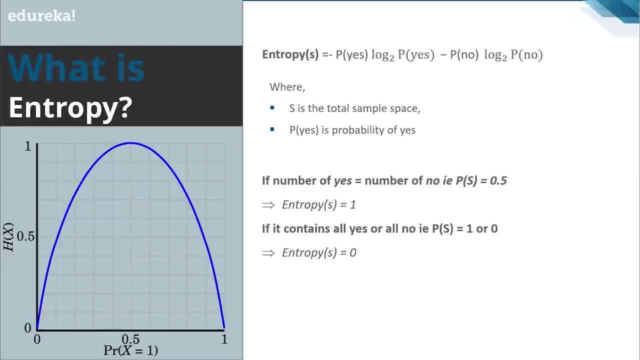 equals 0 or if the data is completely impure. even in that case, the value of impurity will be 0. question like: why is it that the value of entropy is maximum at 0.5 might arise in your mind, right? So let me discuss about that. 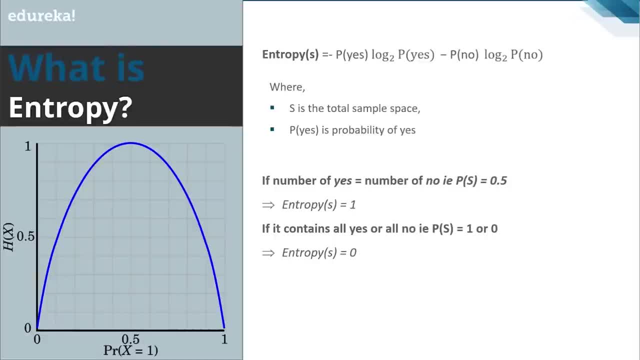 Let me derive it mathematically. as you can see here on the slide, The mathematical formula of entropy is minus of probability of yes. Let's move on and see what this graph has to say mathematically. suppose s is our total sample space and it's divided into two. 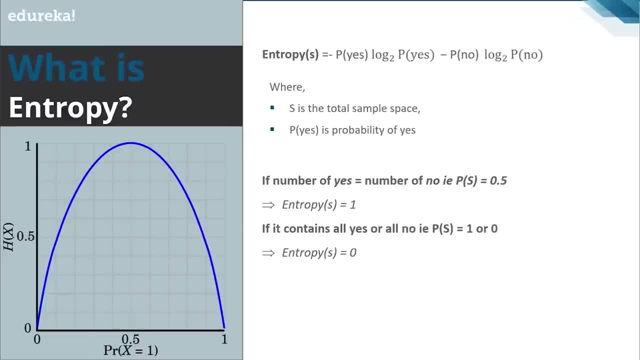 parts, Yes and no, like in our data set, the result for playing was divided into two parts, either yes or no, which we have to predict. either we have to play or not, right? So for that particular case, you can define the formula of: 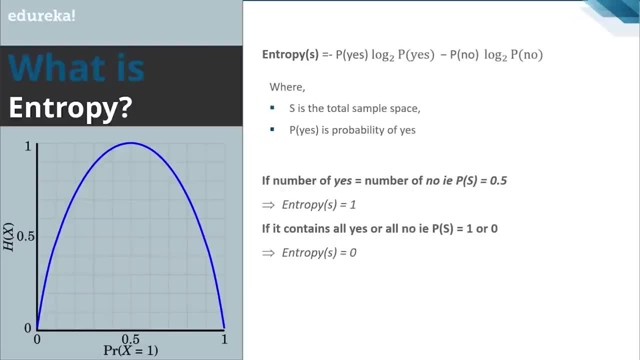 entropy, as entropy of total sample space equals negative of probability of yes multiplied by log of probability of yes with a base Minus probability of no multiplied by log of probability of no with base to where s is your total sample space and P of yes is the probability of yes and P of no is the probability. 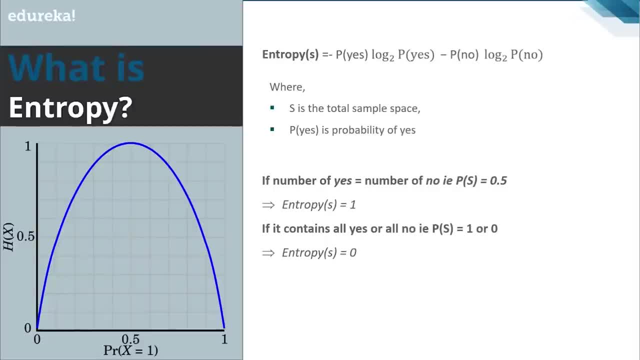 of no. well, if the number of yes equal number of no, that is, probability of s equals 0.5, right, since you have equal number of yes and no. so in that case, value of entropy will be one. just put the value over there. All right, let me just move to the next slide. 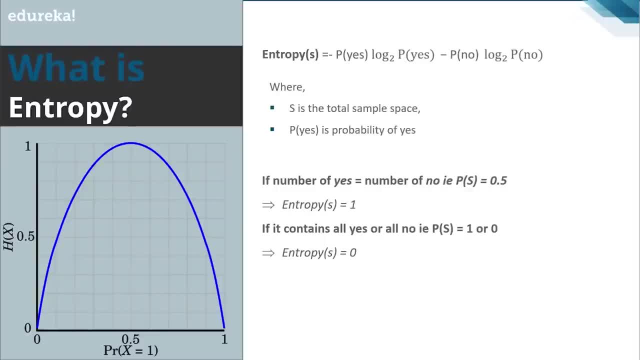 divided into two parts, Either yes or no, which we have to predict. either we have to play or not, right? So for that particular case, you can define the formula of entropy as entropy of total sample space equals negative of probability of yes multiplied by log of probability of yes. 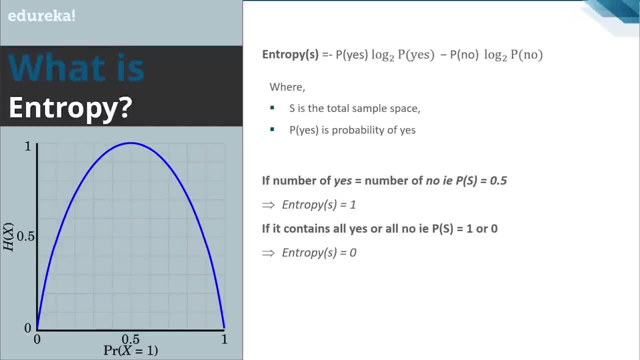 with a base 2 minus probability of no multiplied by log of probability of no. with base 2, where s is your total sample space and P of yes is the probability of yes and P of no is the probability of no. Well, if the Number of yes equal number of no, that is probability of s equals. 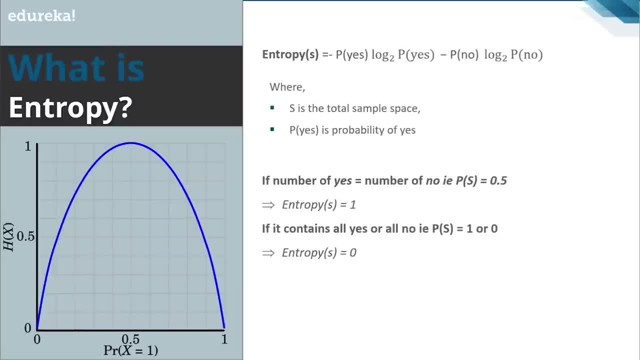 0.5, right, since you have equal number of yes and no. so in that case, value of entropy will be one. just put the value over there. All right, Let me just move to the next slide. I'll show you this, All right. 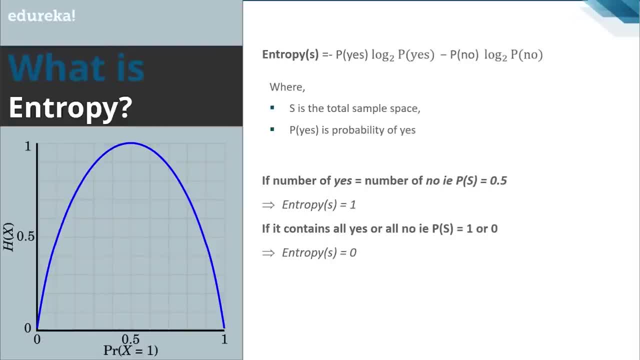 Next is if it contains all yes or all no, that is, probability of a sample space is either 1 or 0, then in that case entropy will be equal to 0.. Let's see it mathematically one by one. So let's start with the first. 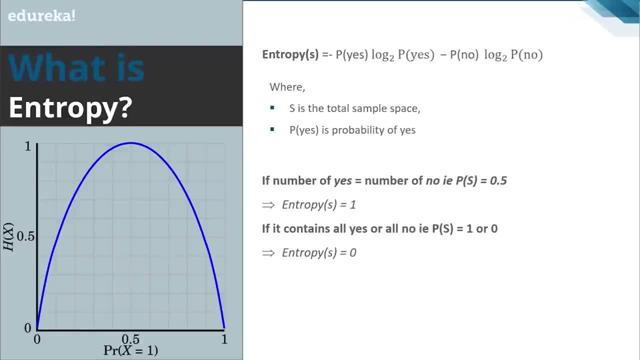 Condition where the probability was 0.5.. So this is our formula for entropy, right? So this is our first case right, which we discussed, that when the probability of yes equal probability of no, that is, in our data set We have equal number of yes and no. 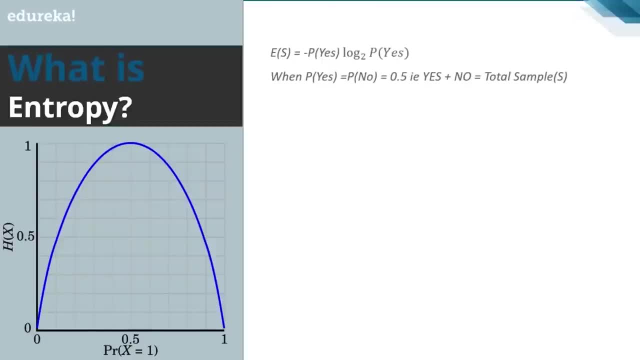 All right. so probability of yes equal probability of no and that equals 0.5. or in other words, you can say that yes plus no equal to total sample space. All right, since the probability is 0.5.. So when you put the values in the formula, you get something. 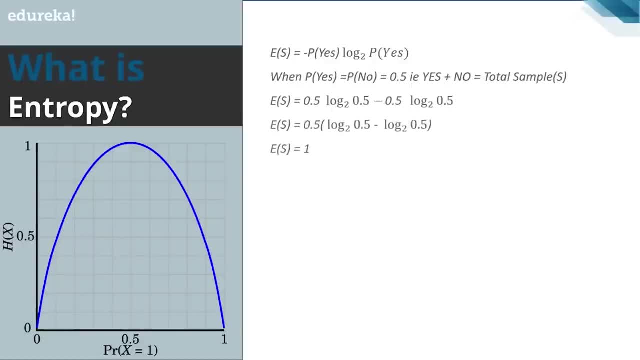 like this and when you calculate it, you'll get the entropy of the total sample space as one. All right, Let's see for the next case. What was the next case? either you have total Yes or you have total no. So if you have total yes, let's see the formula. when we 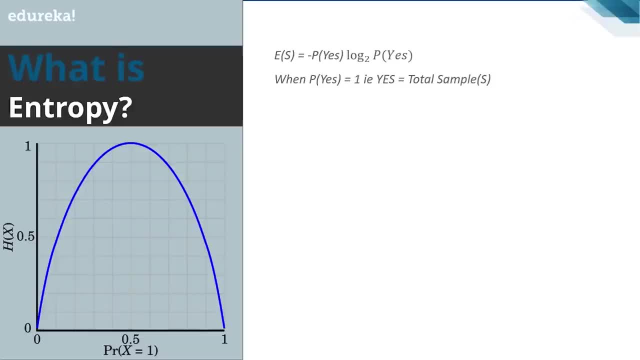 have total Yes, So you have all yes and zero. No fine. So probability of yes equal one and yes as the total sample space. obviously. So in the formula when you put it, Put that thing up, you'll get entropy of sample space equal. 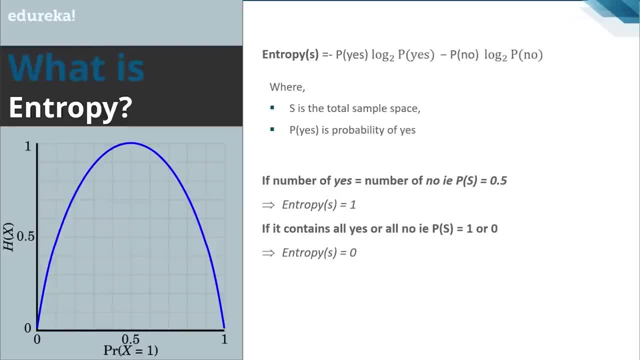 I'll show you this All right. Next is, if it contains all yes or all no- that is, probability of a sample space- is either 1 or 0, then in that case entropy will be equal to 0.. Let's see it mathematically one by one. 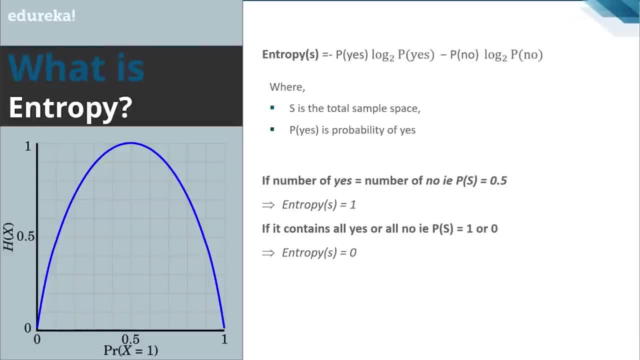 So let's start with the first condition, where the probability was 0.5.. So this is our formula for entropy, right? So this is our first case, right, which we discussed, that when the probability of yes equal probability of no, that is in our data set. 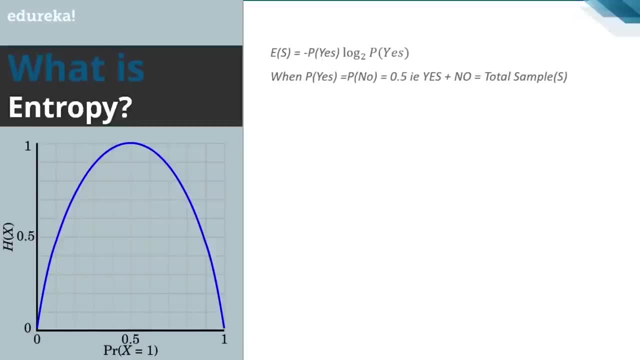 We have equal number of yes and no, All right, so probability of yes equal probability of no, and that equals 0.5. or in other words, you can say that yes plus no equal to total sample space. All right, since the probability is 0.5.. 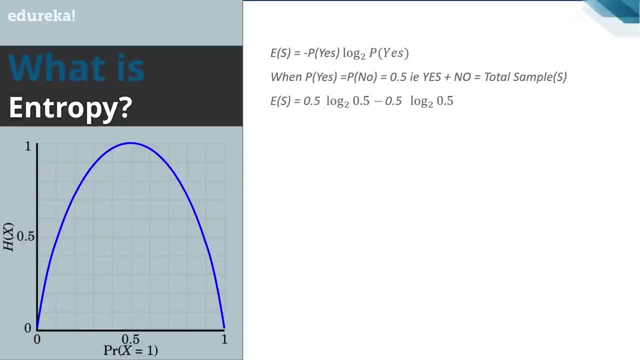 So when you put the values in the formula, you get something like this, and when you calculate it, you'll get the entropy of the total sample space as well. All right, let's see for the next case. What was the next case? either you have total, yes, or you have. 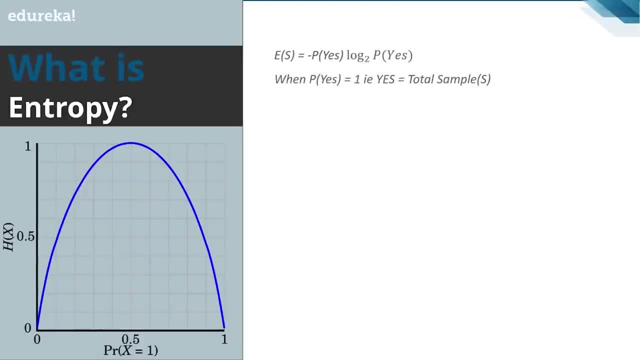 total no. So if you have total yes, let's see the formula when we have total Yes. So you have all yes and 0, no, fine. So probability of yes equal 1 and yes as the total sample space, obviously. so in the formula when you put that thing, 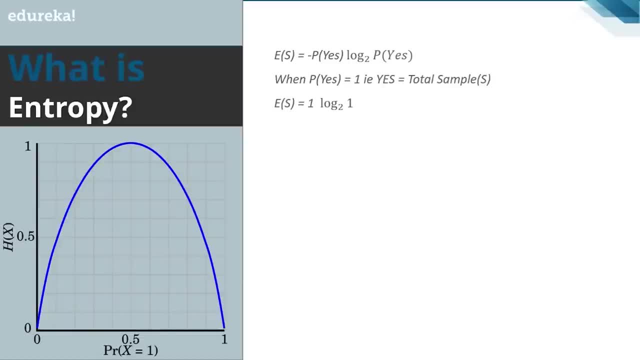 up, you will get entropy of sample space equal negative times of 1 multiplied by log of 1, as the value of log 1 equals 0. So the total thing will result to 0. similarly is the case with no. even in that case you'll get the entropy of total sample. 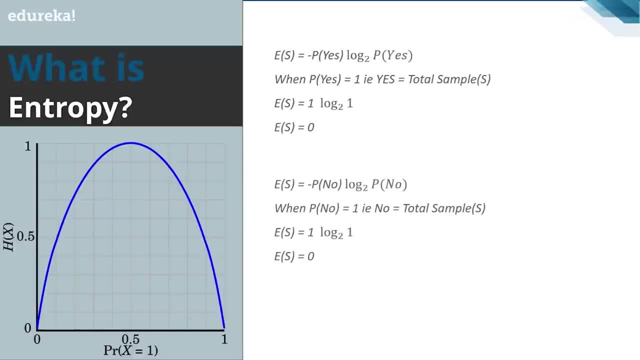 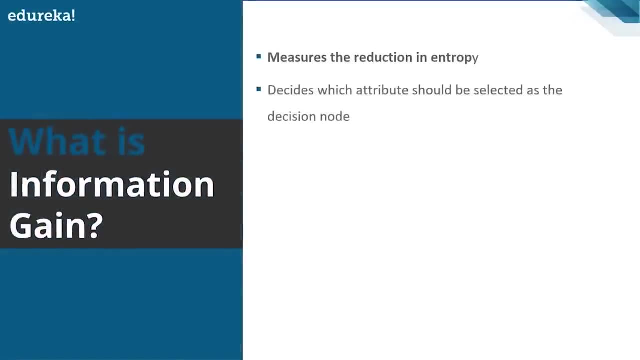 space as 0.. So this was all about entropy. All right. next is, what is information gain? Well, information gain. what it does? it measures the reduction in entropy. It decides which attribute should be selected as the decision node. If s is our total collection, then information gain equals. 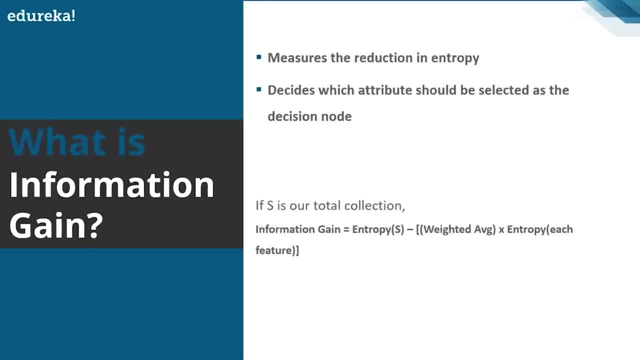 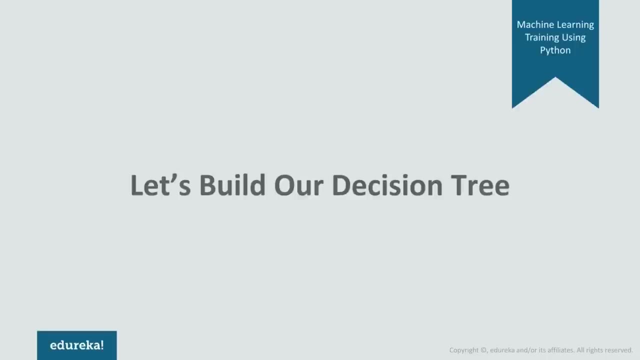 entropy which we calculated just now, that minus weighted average multiplied by entropy of each feature. Don't worry, We'll just see how to calculate it with an example. All right, So let's manually build a decision tree for our data set. So this is our data set, which consists of 14 different. 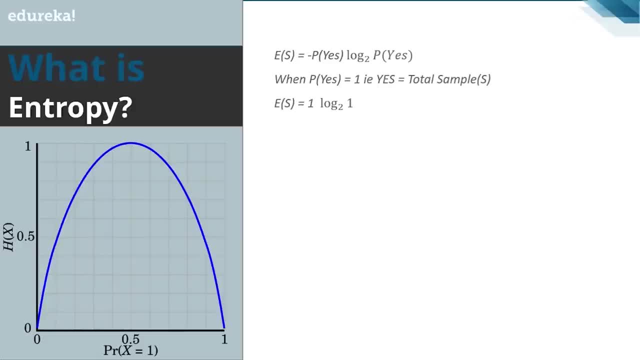 negative times of 1 multiplied by log of 1, as the value of log 1 equals 0. So the total thing will result to 0. similarly is the case with no. even in that case, you'll get the entropy of total sample space as 0. 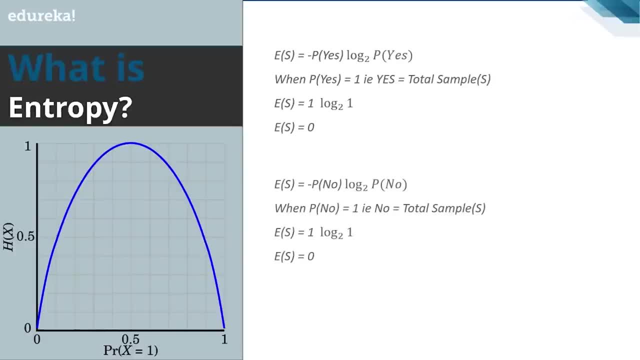 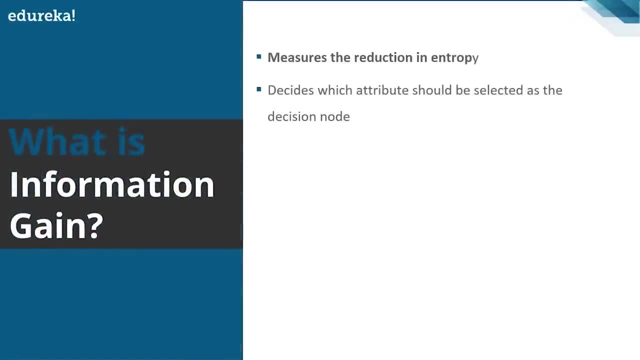 So this was all about entropy, All right. Next is: what is information gain? Well, information gain what it does. it measures the reduction in entropy. It decides which attribute should be selected as the decision node. If s is our total collection, then information gain equals. 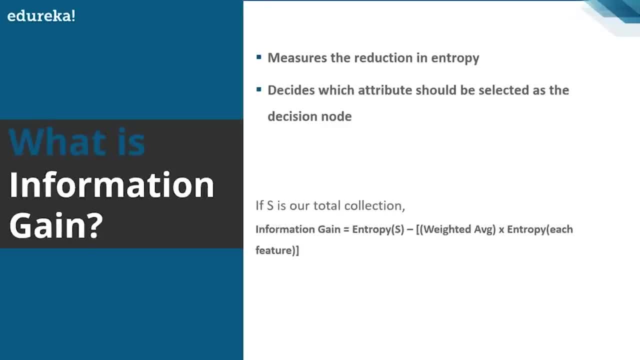 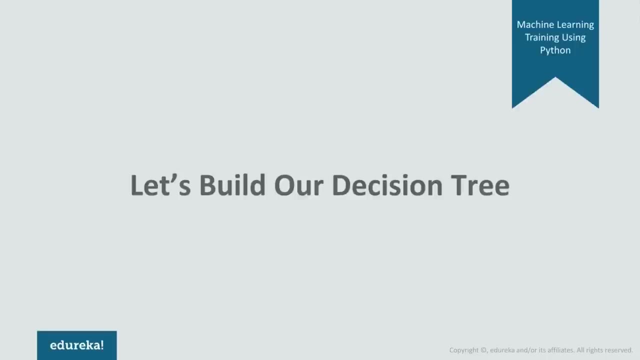 entropy which we calculated just now, that minus weighted average multiplied by entropy of each feature. don't worry, We'll just see how to calculate it with an example. All right, So let's manually build a decision tree for our data set. So this is our data set, which consists of 14 different. 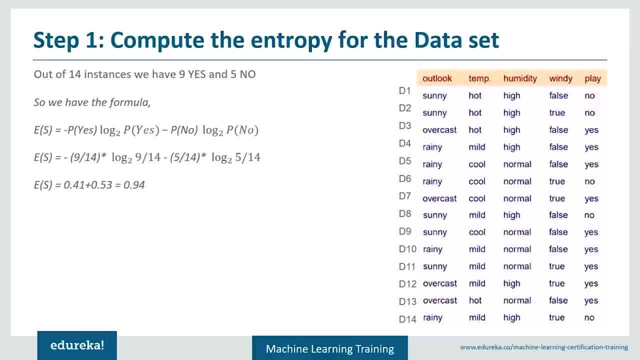 instances, out of which we have nine Yes and five No. all right, So we have the formula for entropy, just put over that since nine years. So total probability of yes equals 9 by 14 and total probability of no equals 5 by 14. and when you put up the value and calculate, 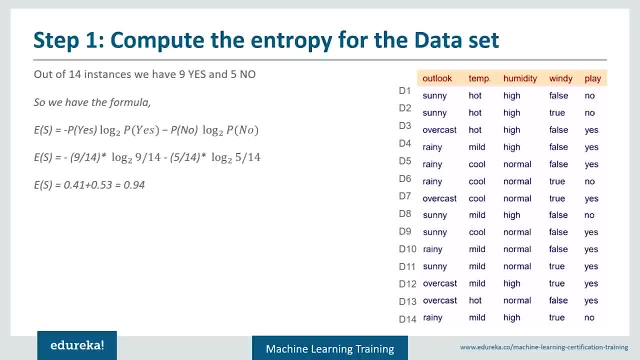 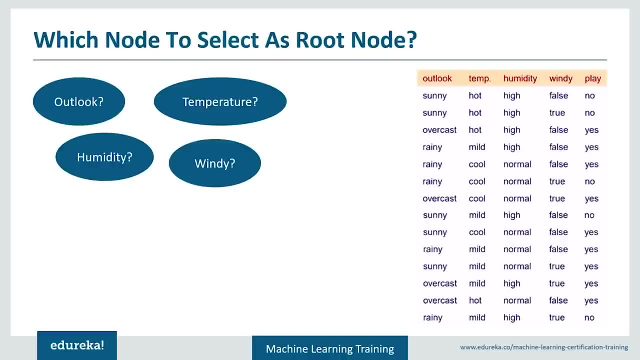 the result. you will get the value of entropy as 0.94.. All right, So this was your first step, that is, compute the entropy for the entire data set. All right, Now you have to select that out of Outlook: temperature, humidity and windy. which of the node should you select as the root? 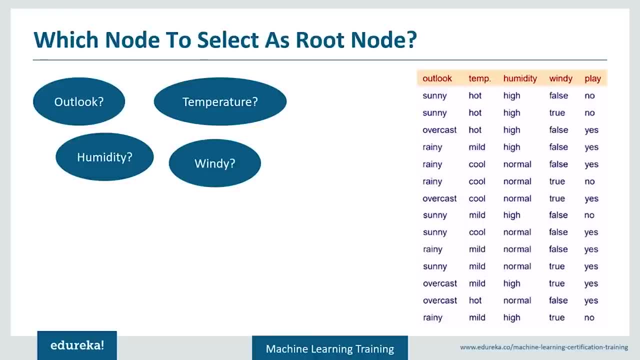 node. Big question, right? How will you decide that this particular node should be chosen at the base node? and on the base of that only I'll be creating the entire tree. I will select that, Let's see. So you have to do it one by one. you have to calculate the. 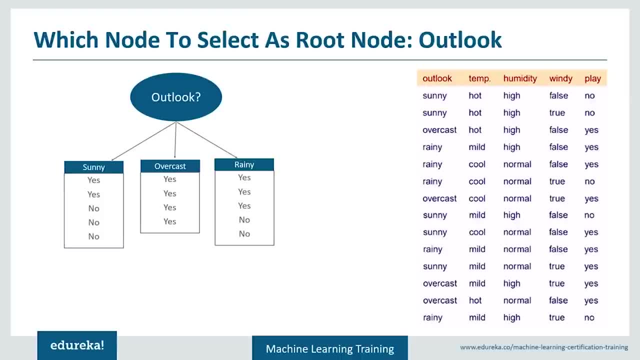 entropy and information gain for all of the different nodes. So starting with Outlook. so Outlook has three different parameters: sunny, overcast and rainy. So first of all, select how many number of yes and no are there. in the case of sunny, like when it is sunny, how many number of 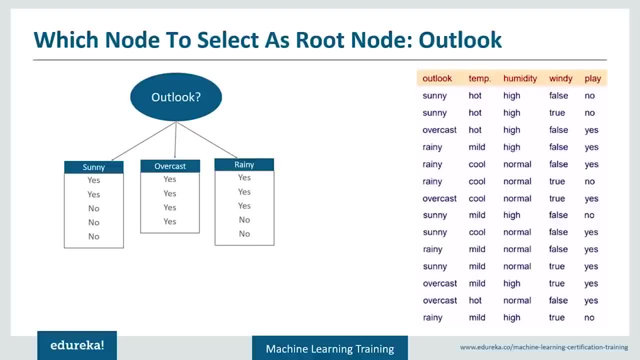 yes, and how many number of no's are there? So in total we have two yes and three no's. in case of sunny, in case of overcast, We have all yes. So if it is overcast, then we'll surely go to play. 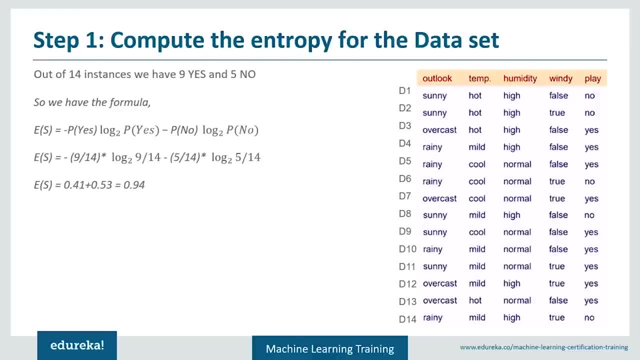 instances, out of which we have nine Yes and five No. all right, So we have the formula for entropy, just put over that since nine years. So total probability of yes equals 9 by 14 and total probability of no equals 5 by 14. and when you put up the value and calculate, 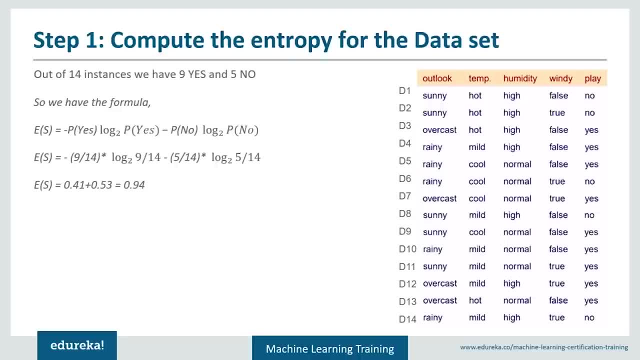 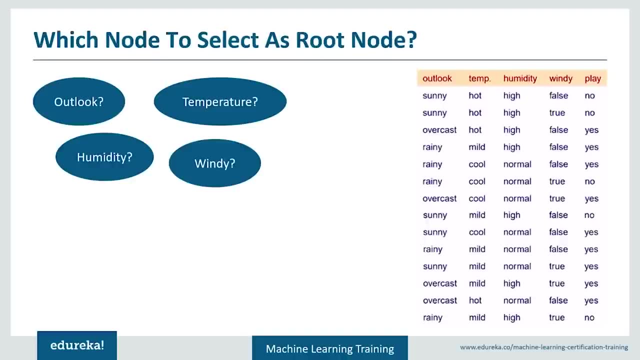 the result. you will get the value of entropy As 0.94.. All right, So this was your first step, that is, compute the entropy for the entire data set. All right, Now you have to select that out of Outlook: temperature, humidity and windy. which of the node should you select as the root? 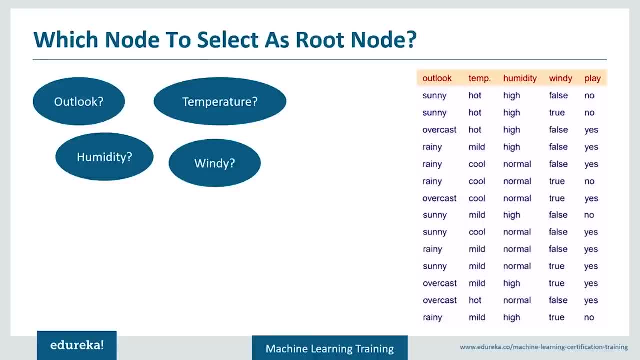 node. big question, right? How will you decide that this particular node should be chosen at the base node? and on the base of that only I'll be creating the entire tree. I will select that, let's see. So you have to do it one by one. you have to calculate the. 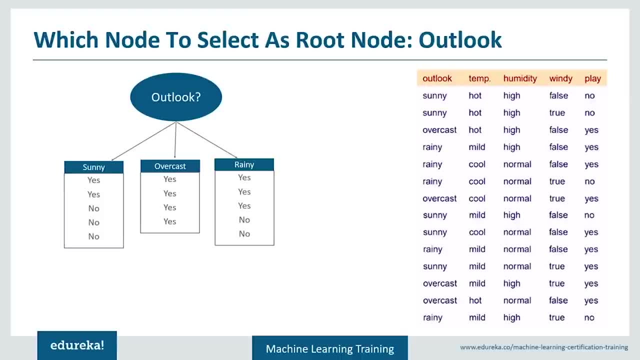 entropy and information gain for all of the different nodes. So starting with Outlook. so Outlook has three different parameters: sunny, overcast and rainy. So first of all, select how many number of yes and no are there. in the case of sunny, like when it is sunny, how many number? 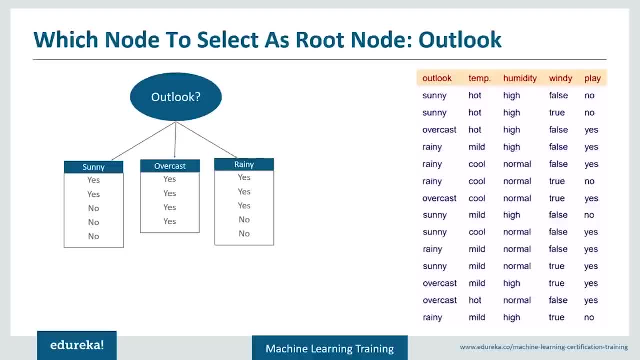 of yes, and how many number of no's are there? So in total we have two years and three no's. in case of sunny, in case of overcast, We have all yes. So if it is overcast, then we'll surely go to play. 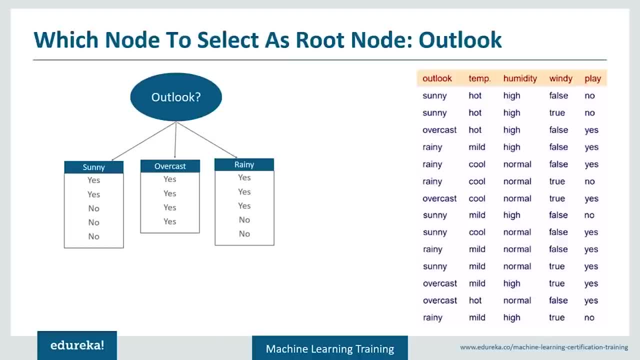 It's like that, All right. and next it is rainy. then total number of yes equal three And total number of no equals two. fine, Next, what we do? we calculate the entropy for each feature. for here We are calculating the entropy when Outlook equals sunny. 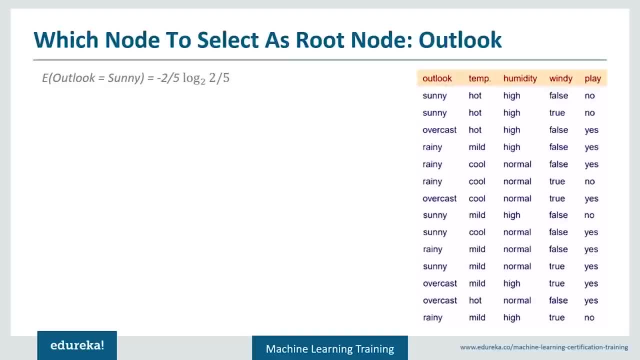 First of all, we are assuming that Outlook is our root node and for that we are calculating the information gain for it. All right. So in order to calculate the information gain, remember the formula. it was entropy of the total sample space minus weighted average, multiplied by entropy of each feature. 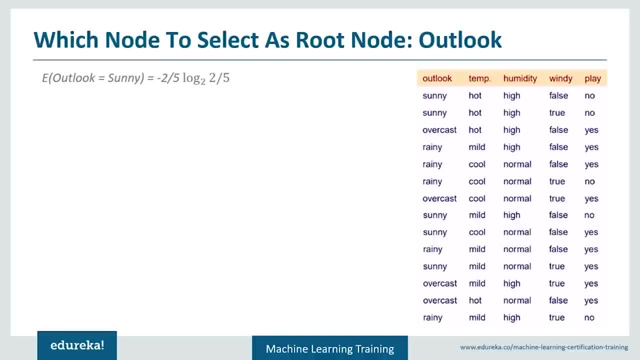 All right. So what we are doing here, we are calculating the entropy of Outlook When it was sunny. so total number of years when it was sunny was two and total number of no, that was three. fine, So let's put up in the formula, since the probability of yes is. 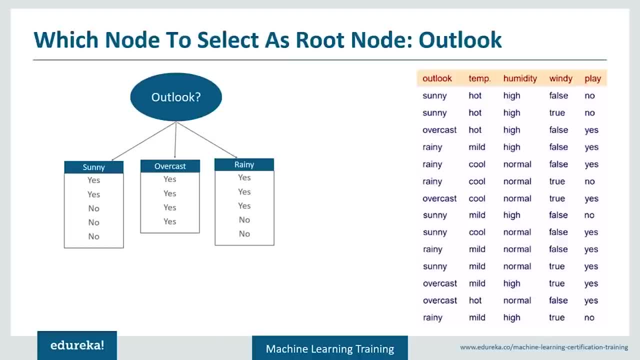 It's like that, All right. and next it is rainy. then total number of yes equal three and total number of no equals two. fine, Next, what we do? we calculate the entropy for each feature. for here We are calculating the entropy when Outlook equals sunny. 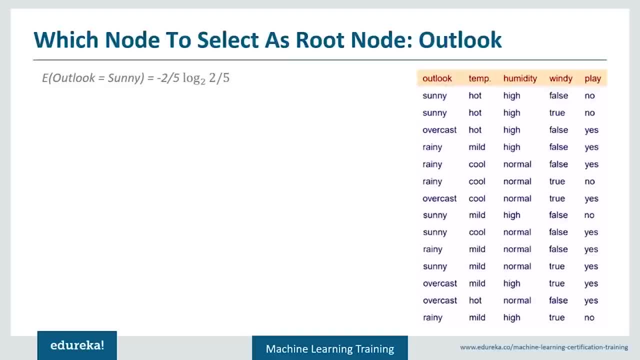 First of all, we are assuming that Outlook is our root node And for that we are calculating the information gain for it. All right. So in order to calculate the information gain, remember the formula. it was entropy of the total sample space minus weighted average, multiplied by entropy of each feature. 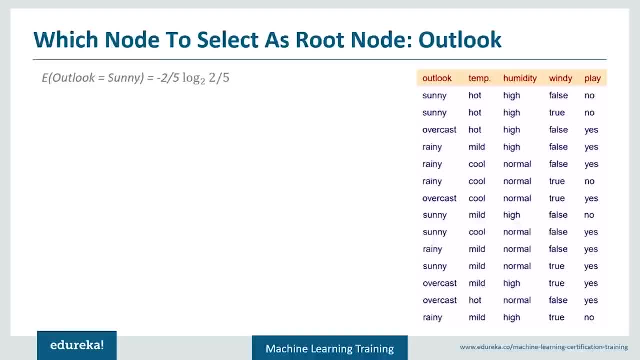 All right. So what we are doing here, we are calculating the entropy of Outlook when it was sunny. So total number of years when it was sunny was two and total number of no, that was three. fine, So let's put up in the formula, since the probability of yes is. 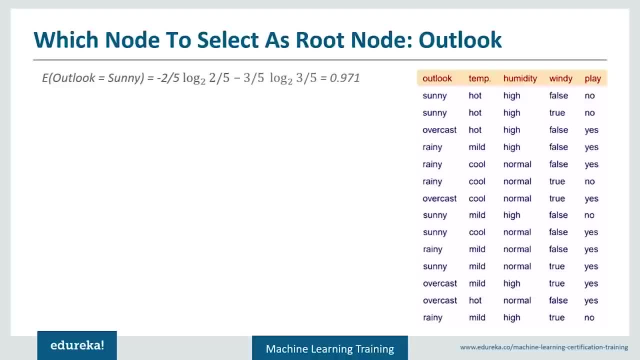 2 by 5, and the probability of no is 3 by 5.. So you will get Something like this: All right, so you are getting the entropy of Sunny as 0.97 one fine. Next, you'll calculate the entropy for overcast. when it was. 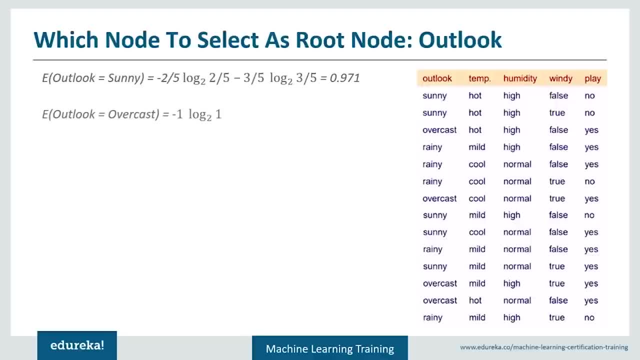 overcast. remember it was all yes, right. So the probability of yes equal one, and when you put over that you'll get the value of entropy as zero. fine, and when it was rainy, rainy has three yes and two no's. so probability of yes in case of Sunny's 3 by 5 and probability of no in case of Sunny. 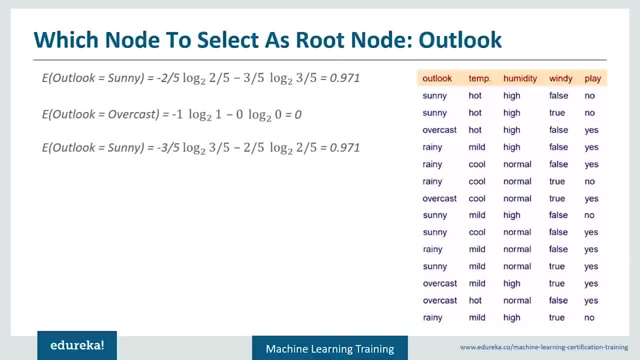 is 2 by 5, and when you add the value of probability of yes and probability of no to the formula, you get the entropy of Sunny as 0.97 one. fine, Now you have to calculate how much information you're getting from Outlook. that equals weighted average. 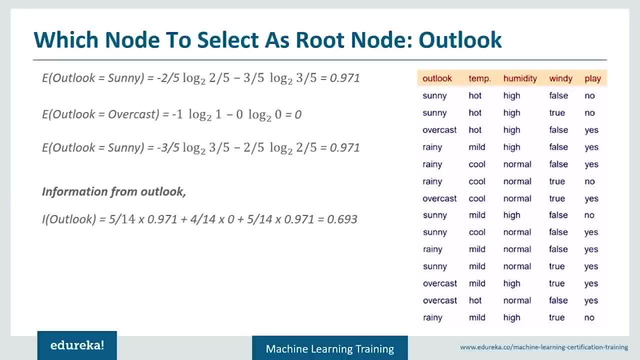 All right. So what was this weighted average? total number of yes and total number of no, fine, So information from Outlook equals 5 by 14. from where does this 5 came over? we are calculating the total number of sample space within that particular Outlook, when it was. 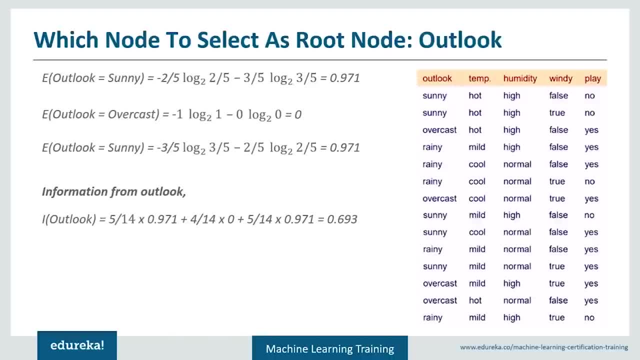 Sunny, right. So in case of Sunny, there was 2 yes and 3 no's. All right, So weighted average for Sunny would be equal to 5 by 14.. All right, since the formula was 5 by 14 multiplied by entropy. 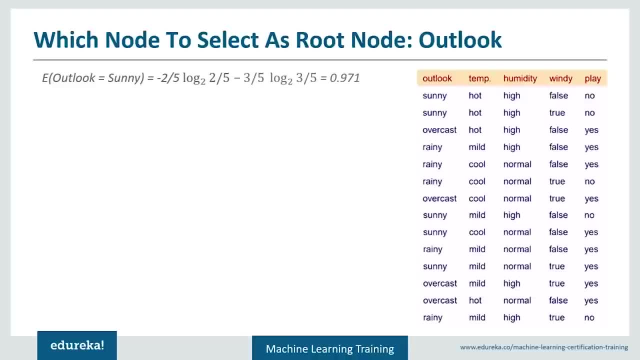 2 by 5 and the probability of no is 3 by 5.. So you will get something like this. All right, so you are getting the entropy of Sunny as 0.971, fine. Next you will calculate the entropy for overcast. when it was. 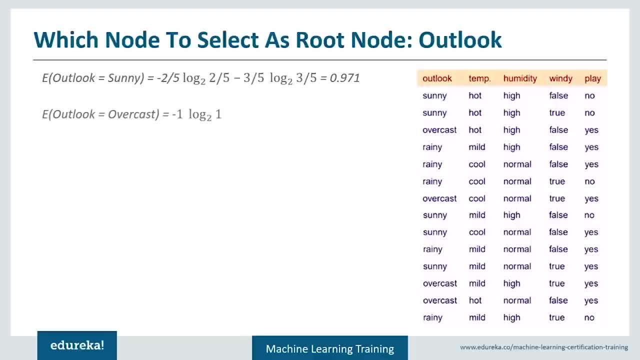 overcast. remember it was all yes, right, So the probability of yes Equal 1 and when you put over that you'll get the value of entropy as 0. fine, and when it was rainy, rainy has 3s and 2 nose, so probability of yes in case of Sunny's 3 by 5 and 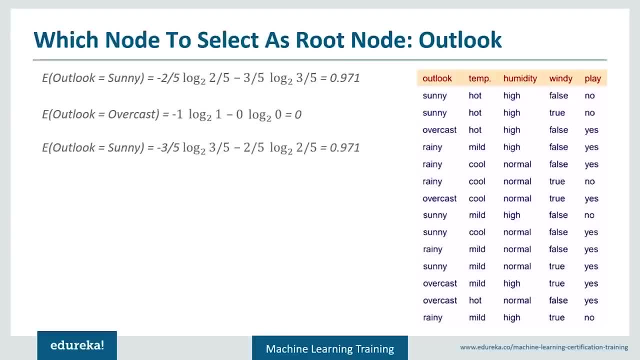 probability of no in case of Sunny is 2 by 5, and when you add the value of probability of yes and probability of no to the formula, you get the entropy of Sunny as 0.971. fine, Now you have to calculate how much information you're getting. 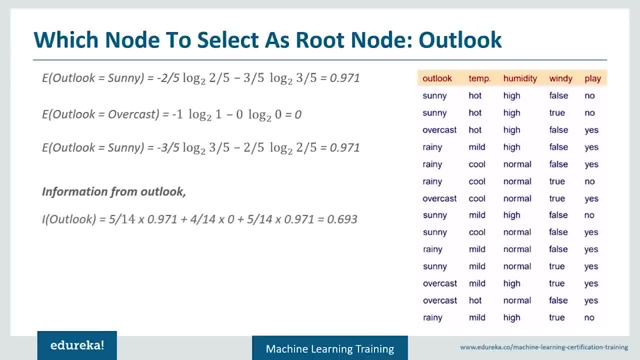 from Outlook that equals weighted average. All right, So what was this weighted Average? total number of yes and total number of no fine, So information from Outlook equals 5 by 14. from where does this 5 came over? We are calculating the total number of sample space within. 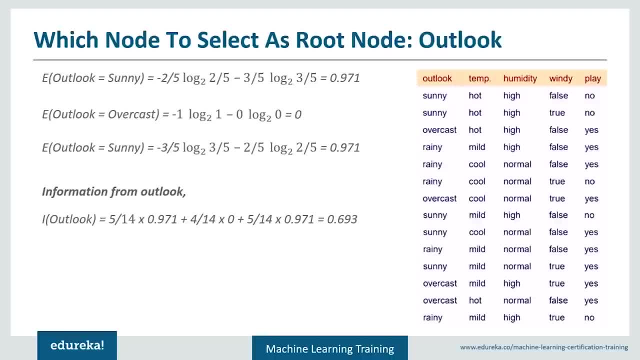 that particular Outlook when it was sunny right. So in case of Sunny there was 2 yes and 3 nose. All right, so weighted average for Sunny would be equal to 5 by 14.. All right, since the formula was 5 by 14 multiplied by entropy. 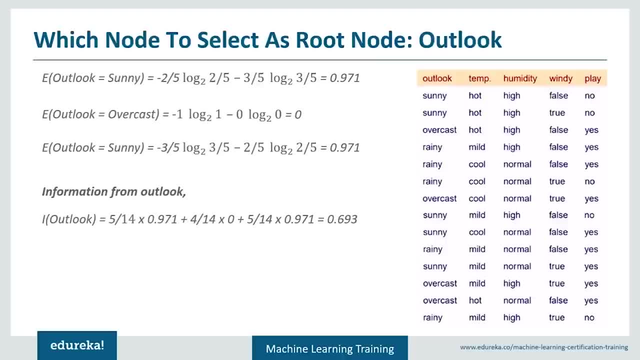 of each feature, All right. So, as calculated, the entropy For Sunny is 0.971, right. So what we'll do will multiply 5 by 14 with 0.971, right? Well, this was a calculation for information when Outlook. 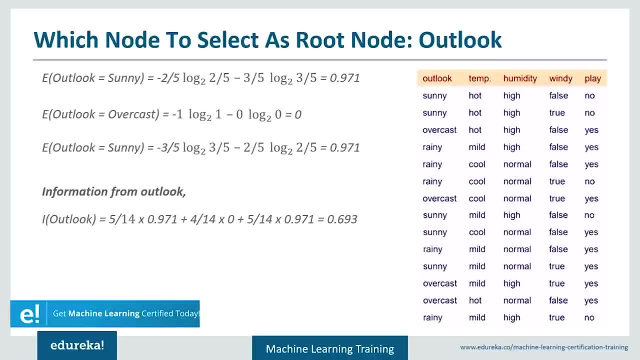 equals Sunny, but Outlook even equals overcast and rainy. for in that case, what we'll do again similarly, will calculate for everything, for overcast and Sunny. for overcast, weighted averages 4 by 14, multiplied by its entropy, that is 0, and for Sunny it is same 5 by 14.. 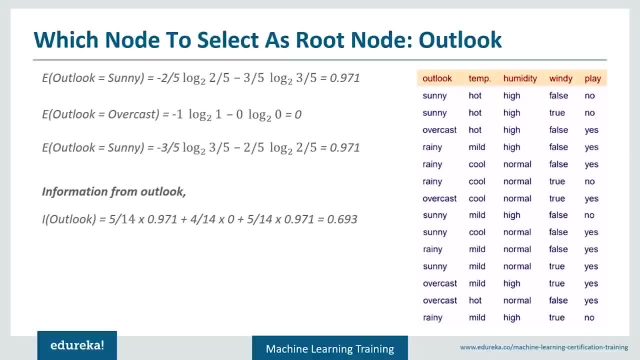 3 yes and 2 nose, multiplied by its entropy, that is 0.971, and finally will take the sum of all of them, which equals to 0.693. right next will calculate the information gained. this, what we did earlier was information taken from Outlook. 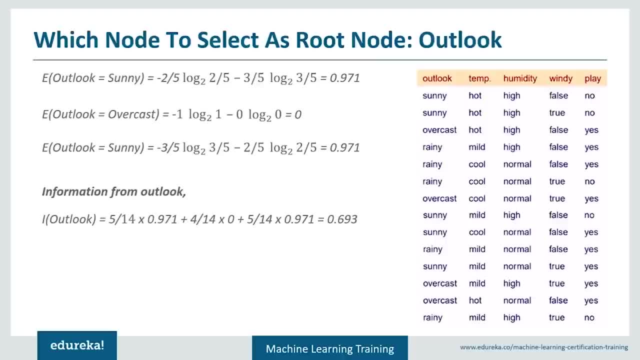 of each feature, All right. So, as calculated, the entropy for Sunny is 0.97 one right. So what we'll do will multiply 5 by 14 with 0.97 one right. Well, this was a calculation for information when Outlook. 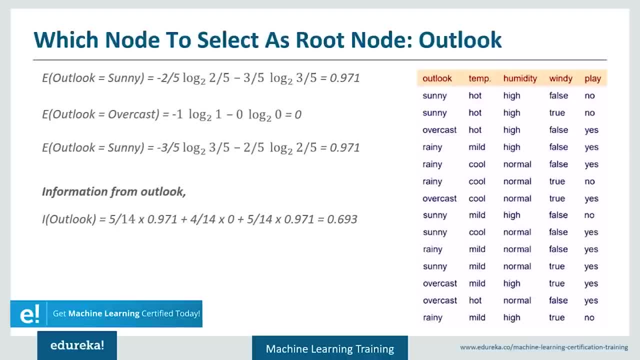 equals Sunny, but Outlook even Even equals overcast and rainy. for in that case, what we'll do again Similarly will calculate for everything, for overcast and Sunny. for overcast, weighted averages 4 by 14, multiplied by its entropy, That is 0, and for Sunny it is same 5 by 14, 3 yes and 2 no's. 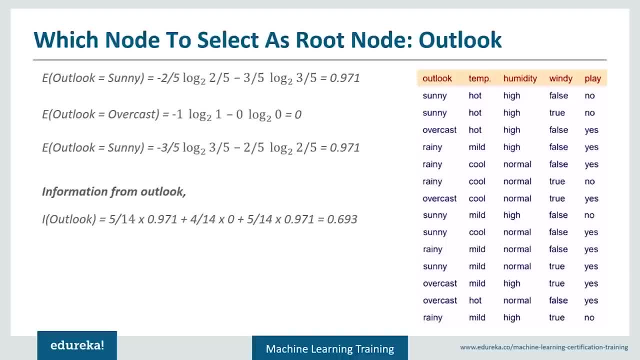 multiplied by its entropy, That is 0.97. when, and finally, will take the sum of all of them, which equals to 0.693. right next will calculate the information gained. This, what we did earlier, was information taken from Outlook. Now we are calculating what is the information we are gaining. 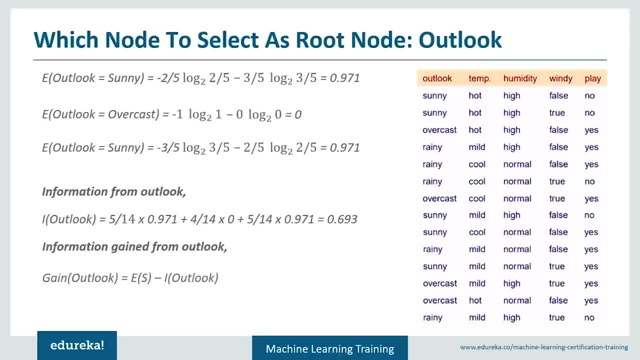 from Outlook. right now this information gain. that equals to total entropy minus the information that is taken from Outlook. All right, so total entropy- we had 0.94, minus information We took from Outlook- is 0.693.. So the value of information gained from Outlook results to: 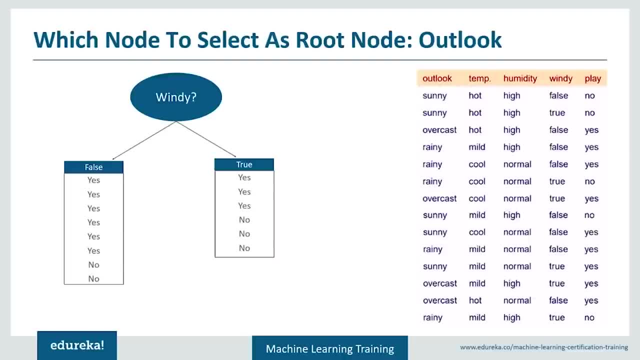 0.247.. All right, So next, what do we have To do? let's assume that Wendy is our root node. So Wendy consists of two parameters, false and true. Let's see how many yes and how many knows are there in case. 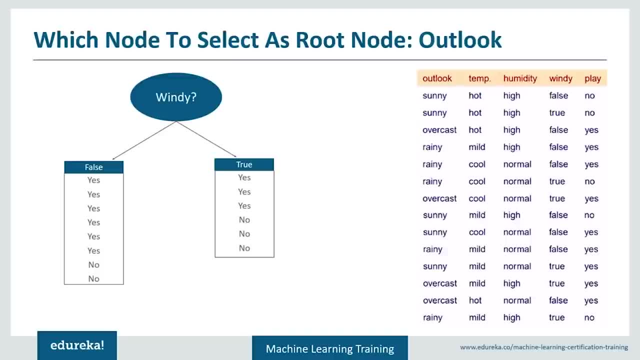 of true and false. So when Wendy has false as its parameter, then in that case it has 6 yes and 2 no's, and when it has true as its parameter, it has 3s and 3 no's. All right, so let's move ahead and similarly calculate the. 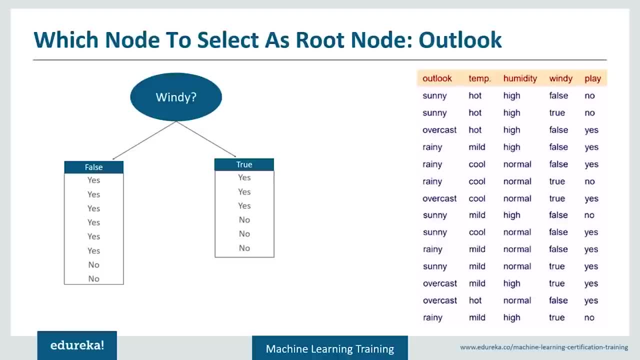 information taken from Wendy and finally, calculate the information gained from Wendy. All right, So first of all, what we'll do will calculate the entropy of each feature, starting with windy, equal true. So, in case of true, we had equal number of yes and equal number. 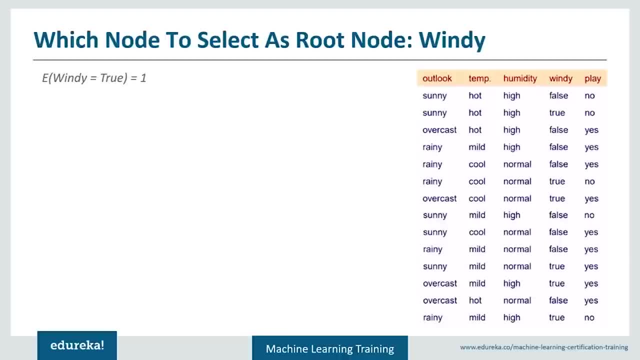 of no will remember the graph when we had the probability as 0.5, as total number of yes equal total number of no and for that case the entropy equals 1, so we can directly write entropy of true when it's windy is 1, as we had already proved it when. 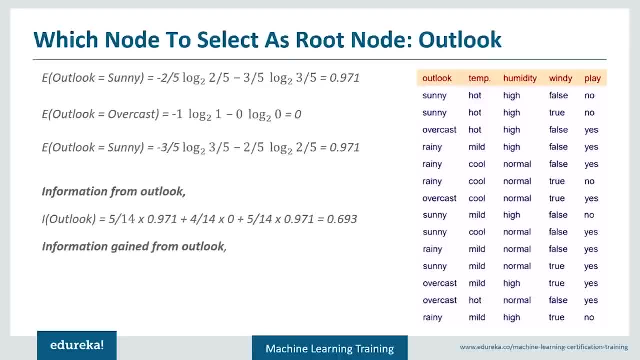 Now we are calculating what is the information we are gaining from Outlook right now. this information gain that equals to total entropy minus the information that is taken from Outlook. All right, So total entropy- we had 0.94, minus information We took from Outlook- is 0.693.. 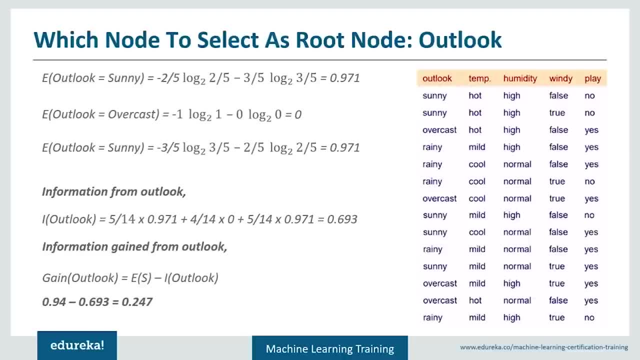 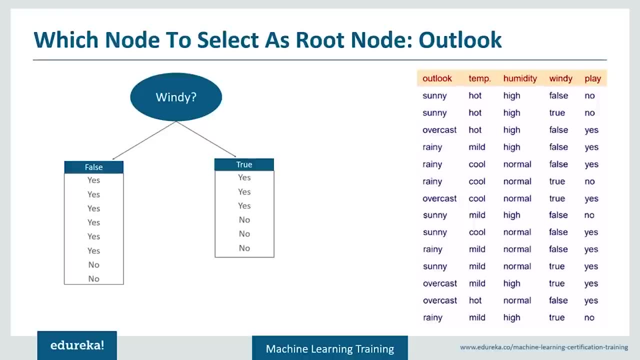 So the value of information gained from Outlook results to 0.247.. All right, So next, what we have to do? Let's assume that Wendy is our root node. So Wendy consists of two parameters, false and true. Let's see how many yes and how many nose are there in case. 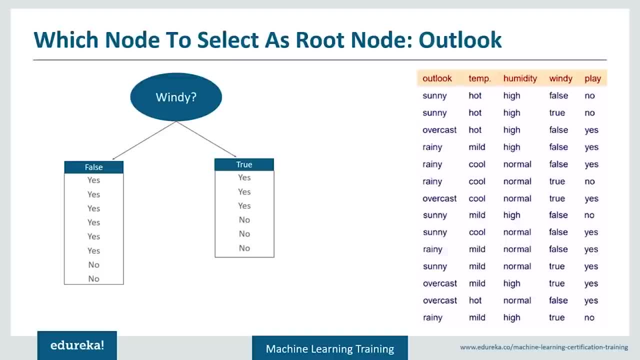 of true and false. So when Wendy has false as its parameter, then in that case it has six yes and two nose, And when it has true as its parameter, it has three years and three knows all right. so let's move ahead. and similarly, 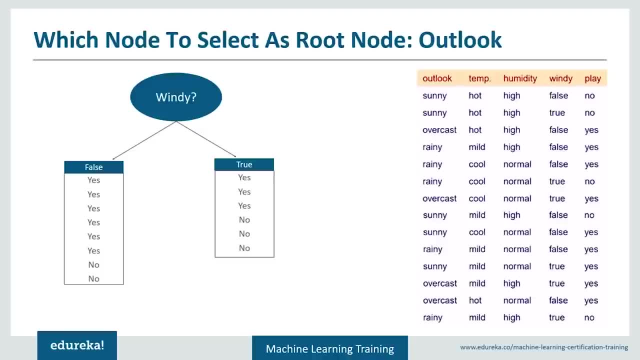 calculate the information taken from Wendy and finally, calculate the information gained from Wendy. All right, So first of all, what we'll do will calculate the entropy of each feature, starting with windy equal true. So, in case of true, we had equal number of yes and equal. 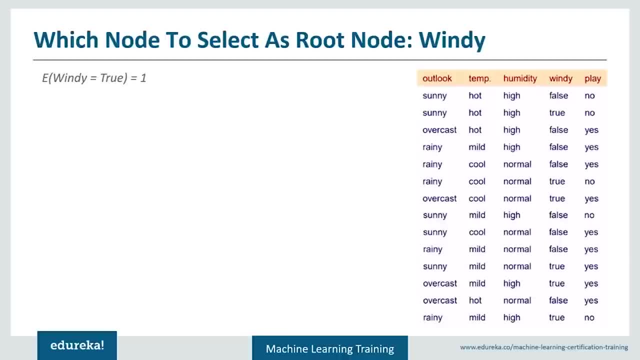 number of no will remember the graph when we had the probability as 0.5, as total number of yes equal total number of no And for that case the entropy equals one. so we can directly write entropy of true- when it's windy is one, as we had already. 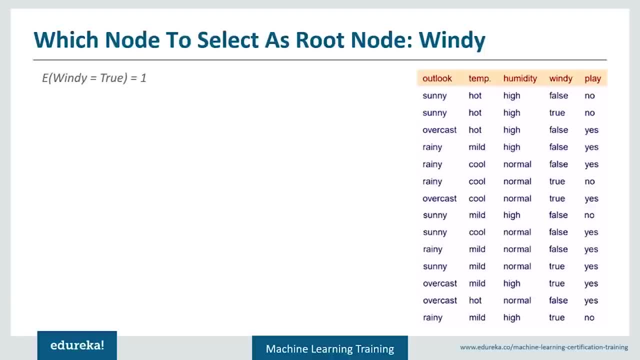 proved it, when probability equals 0.5. The entropy is the maximum that equals to one, All right. Next is entropy of false, when it is Wendy, All right. So, similarly, just put the probability of yes and no in the formula and then calculate the result, since you have six years. 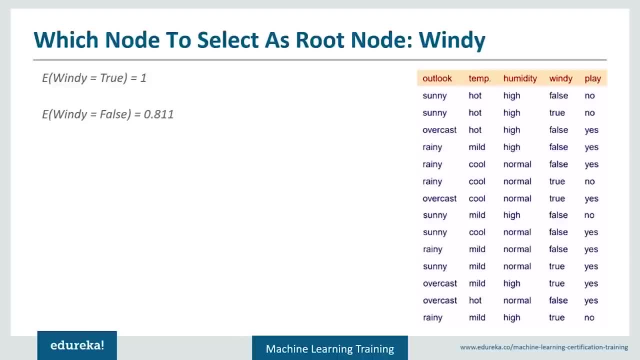 and two nose. So in total you'll get the probability of yes as 6 by 8 and probability of no As 2 by 8.. All right, So when you will calculate it, you will get the entropy of false as 0.811.. 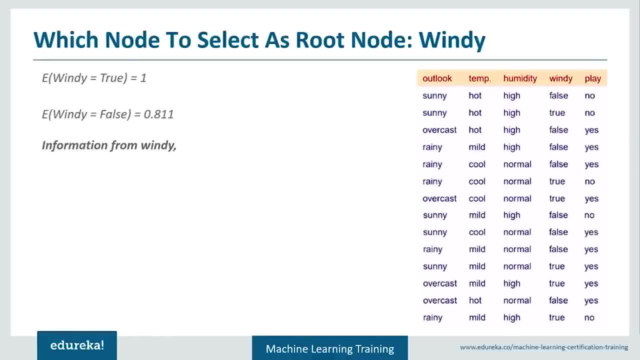 All right, Now let's calculate the information from Wendy. So total information collected from Wendy equals information taken when Wendy equal true, plus information taken when Wendy equal false. So we'll calculate the weighted average for each one of them and then we'll sum it up to finally get the total information. 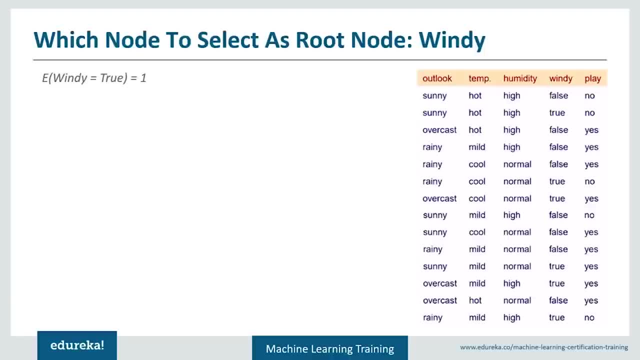 probability equals 0.5.. The entropy is the maximum, that equals to 1.. All right. Next is entropy of false, when it is Wendy, All right. So, similarly, just put the probability of yes and no in the formula and then calculate the result, since you have 6 yes. 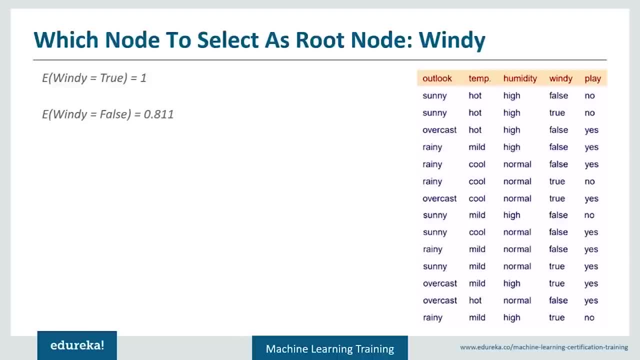 and 2 no's. So in total you'll get the probability of yes as 6 by 8 and probability of no as 2 by 8.. All right, So when you will calculate it, you will get the entropy of false as 0.811.. 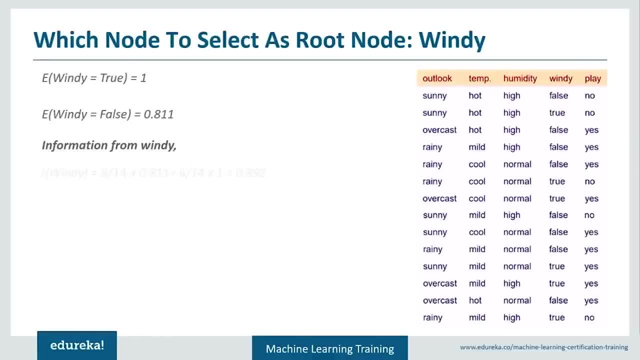 All right, Now let's calculate the information from windy. So total information collected from windy equals information information taken when windy equal true, plus information taken when windy equal false. So we'll calculate the weighted average for each one of them and then we'll sum it up to finally get the total information. 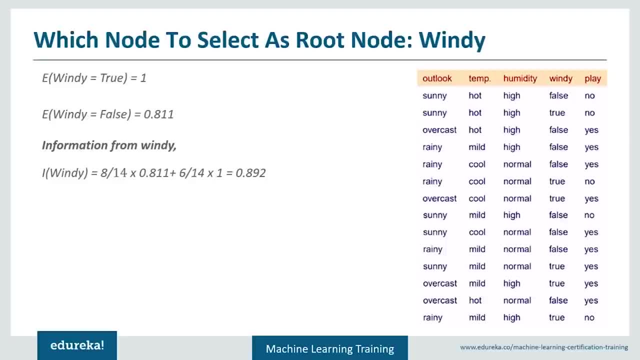 taken from windy. So in this case it equals to 8 by 14 multiplied by 0.811, plus 6 by 14 multiplied by 1.. What is this 8?? It is total number of yes and no in case when windy equals false. 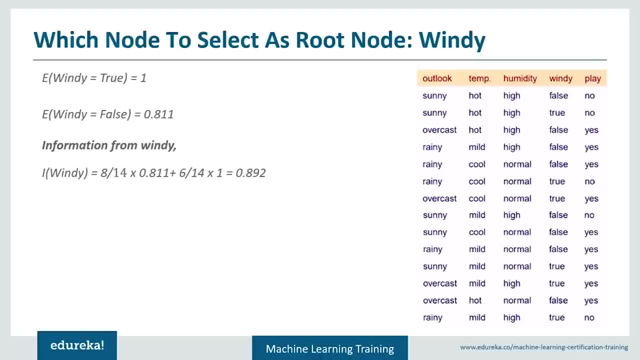 right. So when it was false. so total number of yes, that equals to 6 and total number of no, that equal to 2. That sum ups to 8.. All right, So. that is why the weighted average results to 8 by 14.. 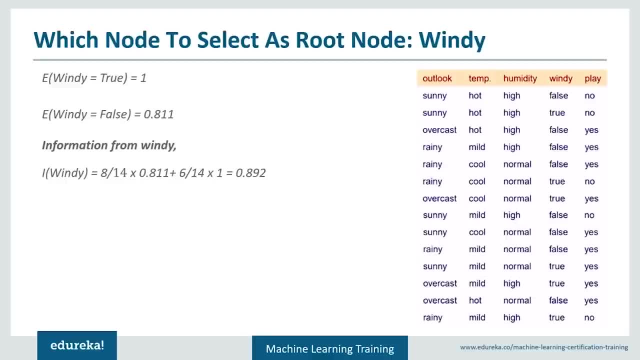 Similarly, information taken when windy equals true equals to 3 plus 3, that is 3.. Yes and 3 no equals 6 divided by total number of sample space. that is 14 x 1. that is entropy of true. All right, so it is 8 by 14 x 0.811 plus 6 by 14 x 1, which. 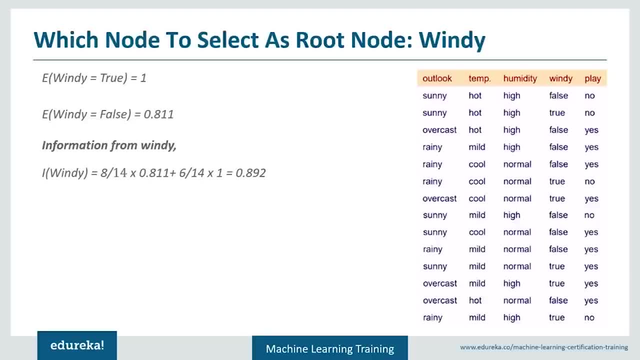 results to 0.892.. This is information taken from windy. All right, Now how much information you are gaining from Wendy? So for that, what you'll do. so total information gained from windy that equals to total entropy minus information taken from windy. 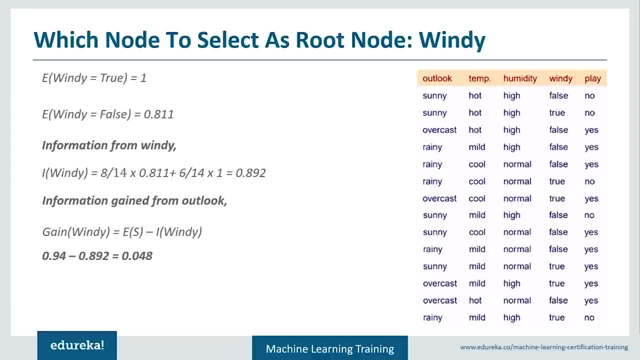 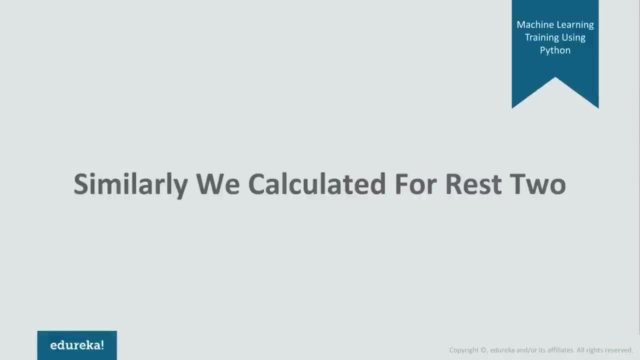 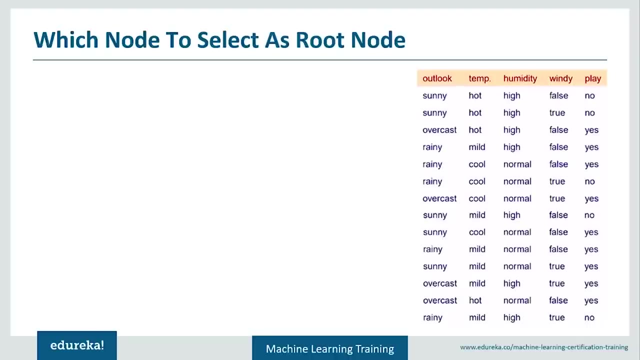 All right, that is 0.94 minus 0.892. that equals to 0.048.. So 0.048 is the information gained from windy. All right. Similarly, we calculated for the rest to all right. So for Outlook, as you can see, the information was 0.693. 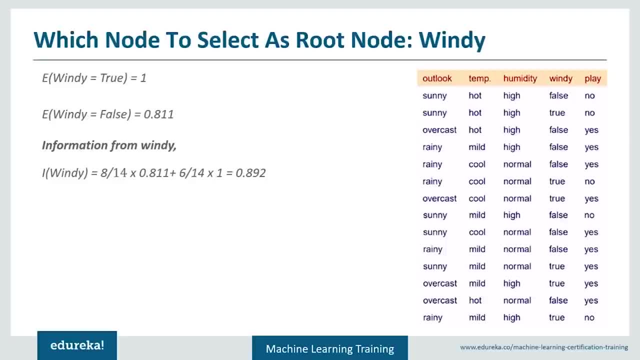 taken from Wendy. So in this case it equals to 8 by 14 multiplied by 0.811.. Plus 6 by 14 multiplied by 1.. What is this 8? 8 is total number of yes and no in case when. 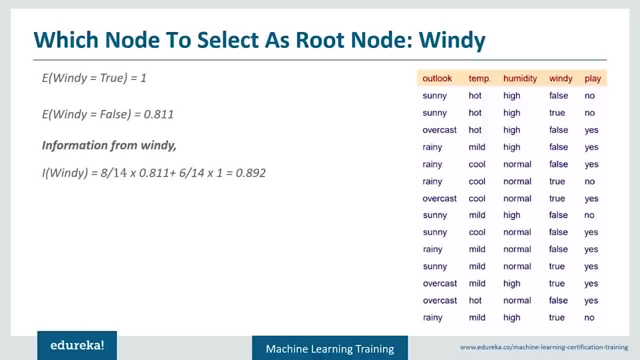 Wendy, equals false right. So when it was false. so total number of yes that equals to 6 and total number of no that equal to 2, that sum ups to 8.. All right, So that is why the weighted average results to 8 by 14.. 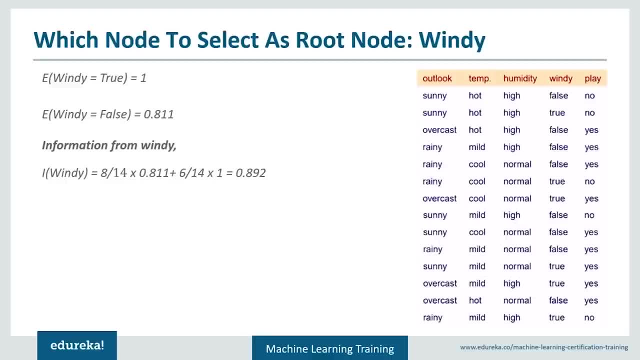 Similarly, information taken when Wendy equals true equals to 3 plus 3, that is, 3 yes and 3 no equals 6 divided by total number of sample space. That is 14 multiplied by One. that is entropy of true. All right, so it is 8 by 14 multiplied by 0.811 plus 6 by 14. 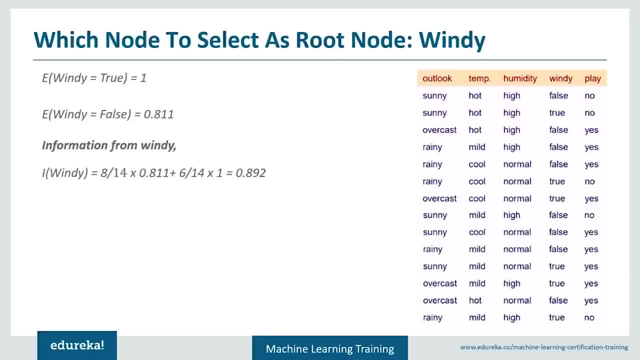 multiplied by 1, which results to 0.892.. This is information taken from Wendy. All right, Now how much information you are gaining from Wendy. So for that, what you'll do. so total information gained from Wendy that equals to total entropy minus information taken. 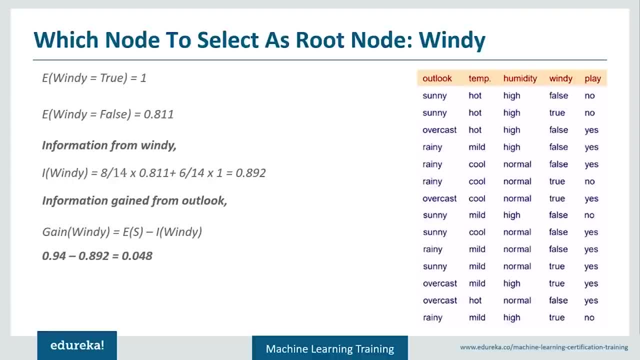 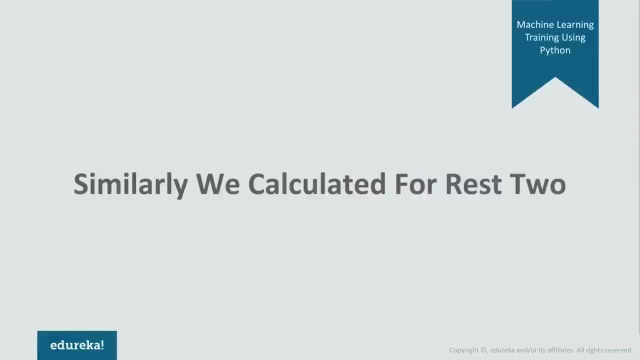 from Wendy All right. that is 0.94 minus 0.892. that equals to 0.048.. So 0.048 is the information gained from Wendy All right. Similarly, we calculated for the rest to all right. So for Outlook, as you can see, the information was 0.693. 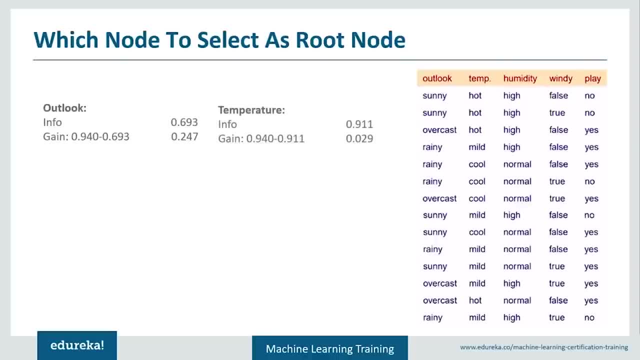 and its information gain was 0.247. in case of temperature, The information was around 0.911 and the information gain that was equal to 0.029. in case of humidity, the information gain was 0.2.. 152 and in the case of Wendy, the information gain was 0.048.. 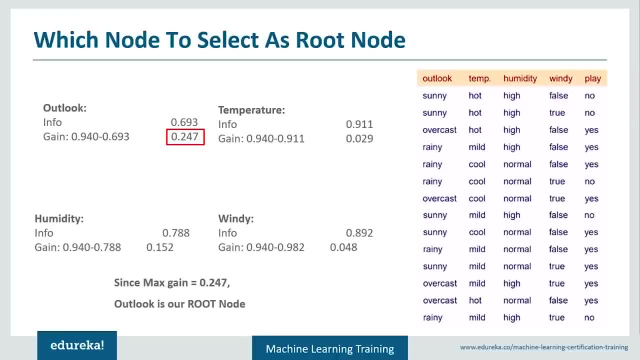 So what we'll do will select the attribute with the maximum mode. fine, Now we are selected Outlook as our root node, and it is further subdivided into three different parts: sunny, overcast and rain. So in case of overcast, we have seen that it consists of all. 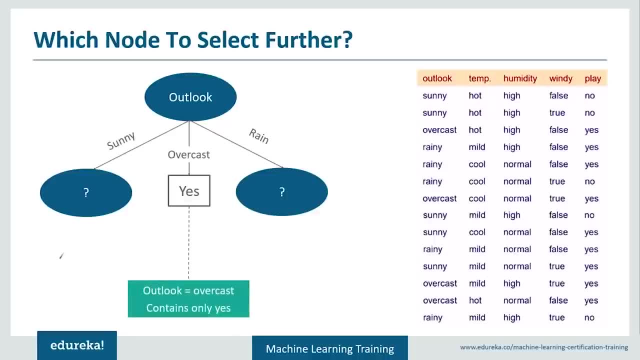 yes, so we can consider it as a leaf node, But in case of sunny and rainy it's doubtful, as it consists of both Yes and both No. So you need to recalculate the things right again for this node. You have to recalculate the things. 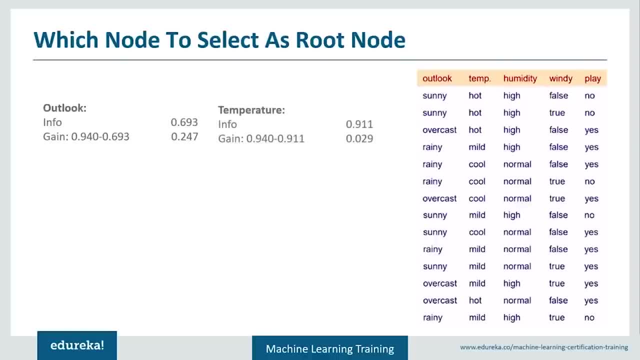 and its information gain was 0.247. in case of temperature, The information was around 0.911 and the information gain that was equal to 0.029. in case of humidity, the information gain was 0.152 and in the case of windy, the information gain was 0.048.. 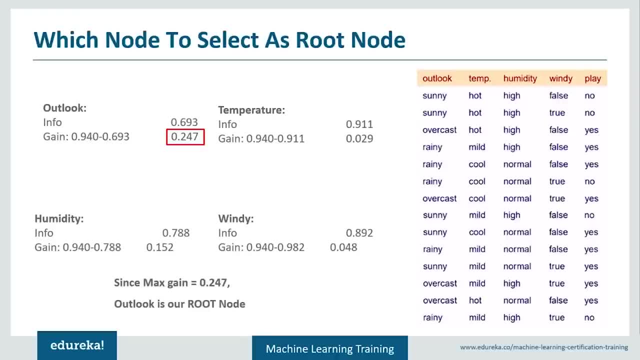 So what we'll do will select the attribute with the maximum mode. fine, Now we are selected Outlook as our root node, And it is further subdivided into three different parts: sunny, overcast and rain. So in case of overcast, we have seen that it consists of all. 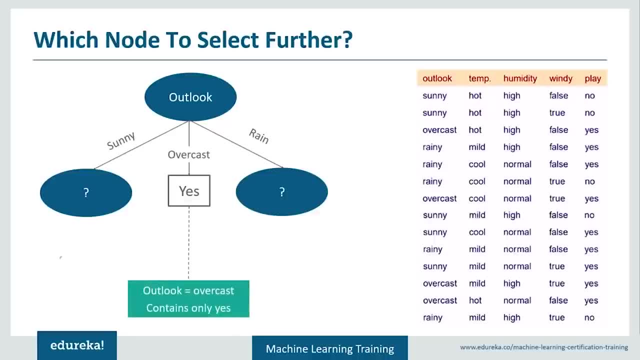 yes, so we can consider it as a leaf node, But in case of sunny and rainy it's doubtful, as it consists of both Yes and both No. so you need to recalculate the things right again for this node. You have to recalculate the things. 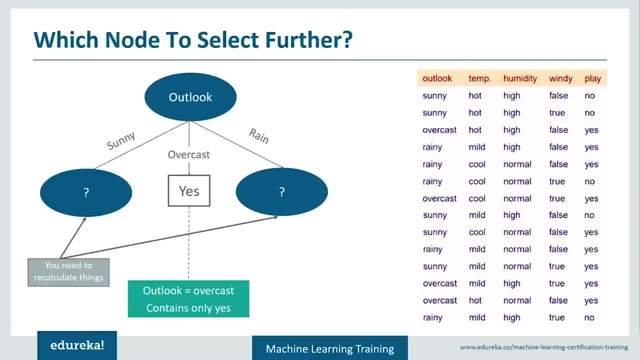 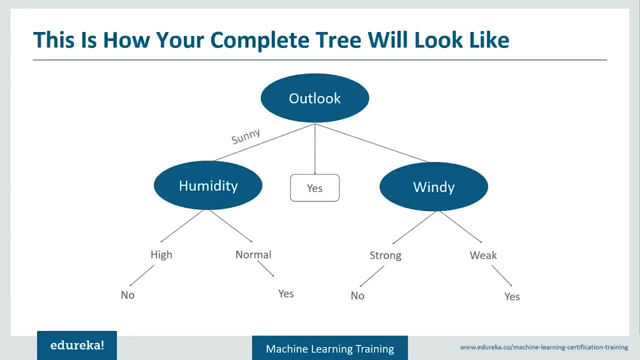 All right, you have to again select the attribute, which is having the maximum information gain. All right, So there's how your complete tree will look Like a light. So let's see when you can play. so you can play when Outlook is overcast. 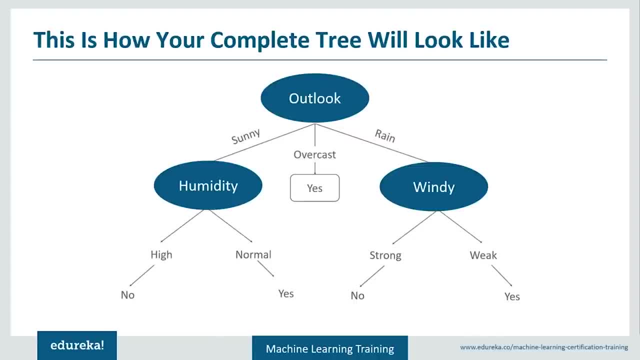 All right, in that case you can always play. if the Outlook is sunny, You will further drill down to check the humidity condition. All right, if the humidity is normal, then you will play. if the humidity is high, then you won't play. right when the 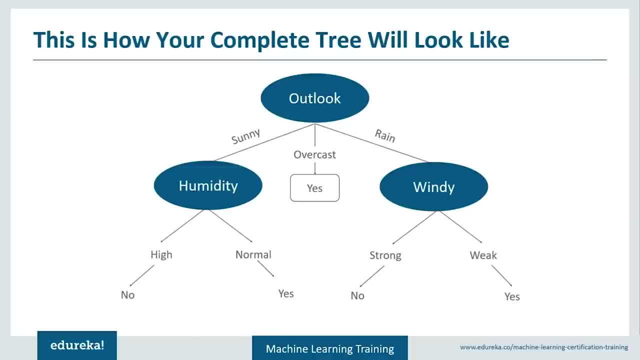 Outlook predicts that it's rainy, then further you'll check whether it's windy or not. If it has a weak wind, then you'll go and opt for play, But if it has strong wind then you won't play right. So this is how your entire decision tree would look. 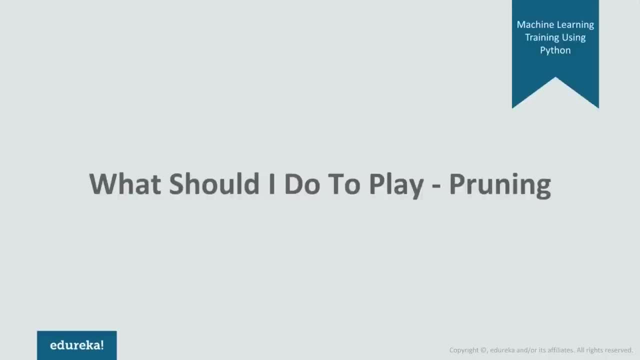 Like at the end. Now comes the concept of pruning. says that: what should I do to play? Well, you have to do pruning. pruning will decide how you will play. What is this pruning? Well, this pruning is nothing but cutting down the nodes in. 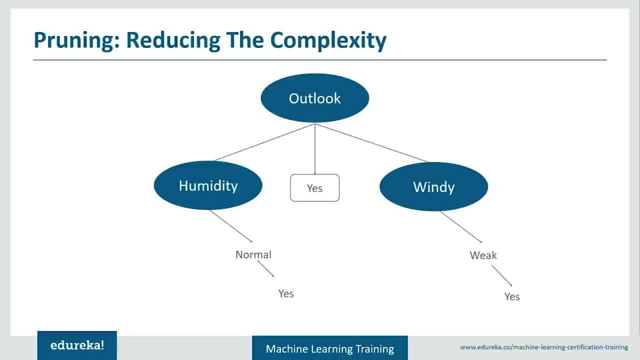 order to get the optimal solution, All right. So what pruning does? it reduces the complexity, All right, as here. you can see on the screen that it's showing only the result for years, That is, it's showing all the result, which says that you can. 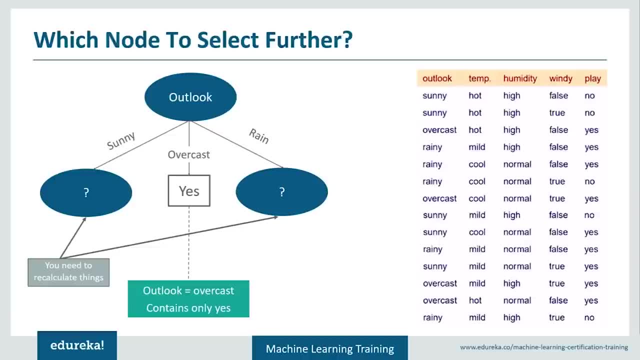 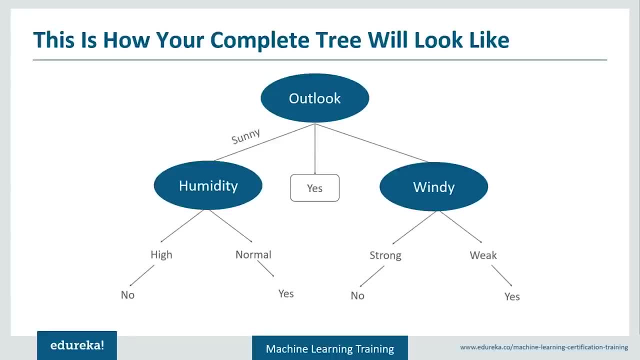 All right, you have to again select the attribute, which is having the maximum information gain. All right, So there's how your complete tree will look like. All right, So let's see when you can play. so you can play when Outlook is overcast. 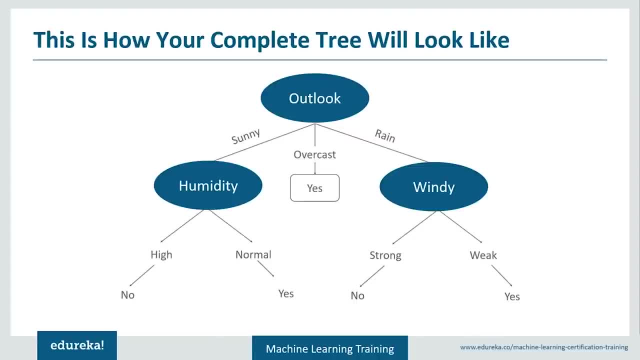 All right, In that case you can always play. if the Outlook is sunny, You will further drill down to check the humidity condition. All right, if the humidity is normal, then you will play. if the humidity is high, Then you won't play. 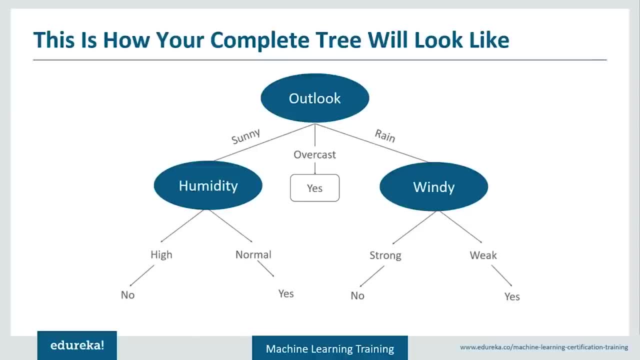 Right when the Outlook predicts that it's rainy, then further you'll check whether it's windy or not. If it has a weak wind then you'll go and opt for play, But if it has strong wind then you won't play. 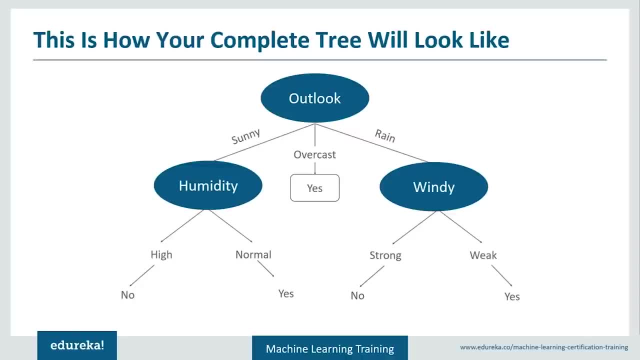 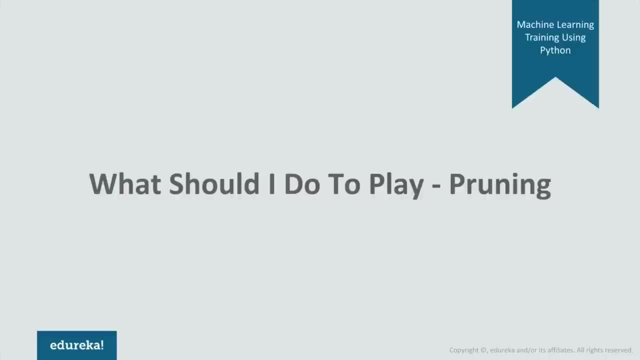 Right. So this is how your entire decision tree would look like at the end. Now comes the concept of pruning. says that: what should I do to play? Well, you have to do pruning. pruning will decide how you will play. What is this pruning? 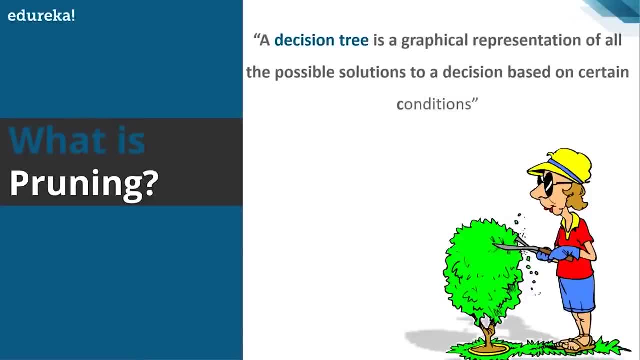 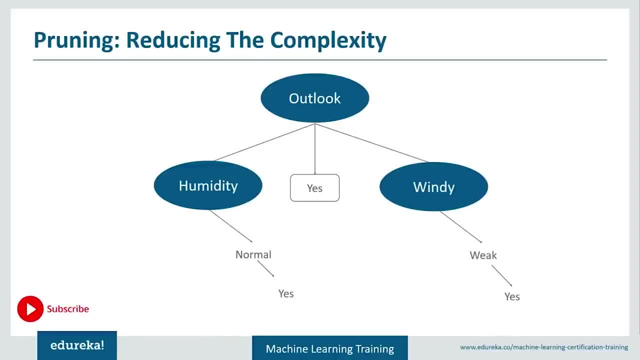 Well, this pruning is nothing but cutting down the nodes in order to get the optimal solution, All right. So what pruning does? it reduces the complexity, All right, as here you can see on the screen that it's showing only the result for years. 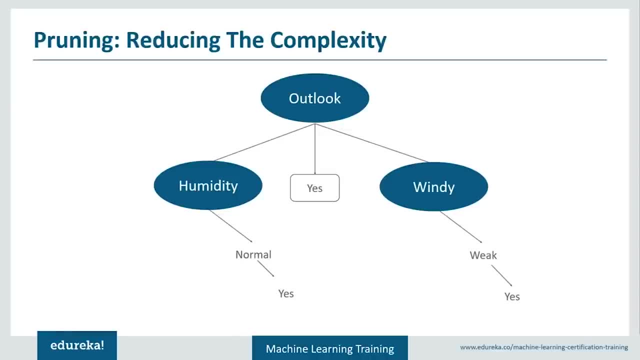 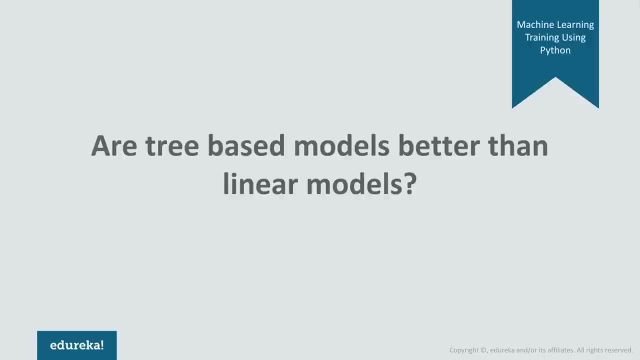 That is it showing all the result which says that you can play. All right, Before we drill down to a practical session, a common question might come in your mind. You might think that a tree based model better than linear model. right, You can think like: if I can use a logistic regression for 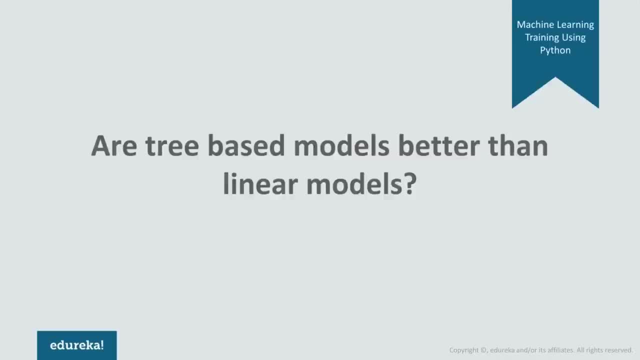 classification problem and linear regression. for regression problem, then why there is a need to use the tree? Well, many of us have this question in their mind and well, there's a valid question to will. actually, as I said earlier, you can use any algorithm. 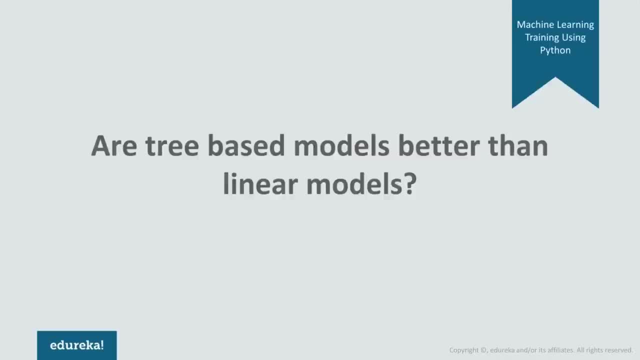 It depends on the type of problem you're solving. Let's look at some key factor which will help you to decide which algorithm to use and when. so the first point being if the relationship between dependent and independent variable is well approximated by a linear model. 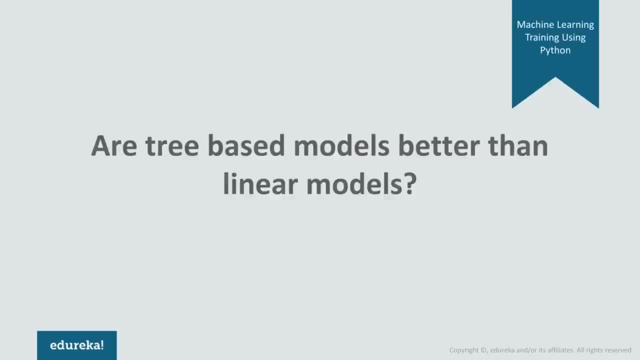 Then linear regression will outperform tree based model. second case: if there is a high non-linearity and complex relationship between dependent and independent variables, a tree model will outperform a classical regression model. and third case: if you need to build a model which is easy. 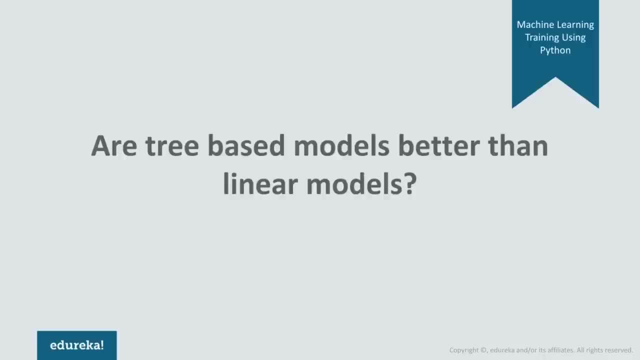 play All right. Before we drill down to a practical session, A common question might come in your mind. You might think that a tree based model better than linear model. right, You can think like: if I can use a logistic regression for classification problem and linear regression for regression? 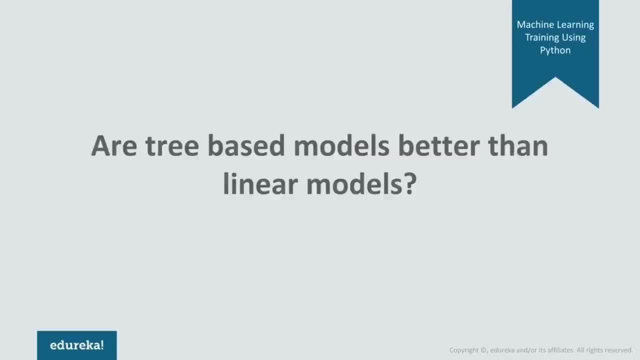 problem, then why there is a need to use the tree. Well, many of us have this question in their mind, and well, there's a valid question too. Well, actually, as I said earlier, you can use any algorithm. It depends on the type of problem you're solving. 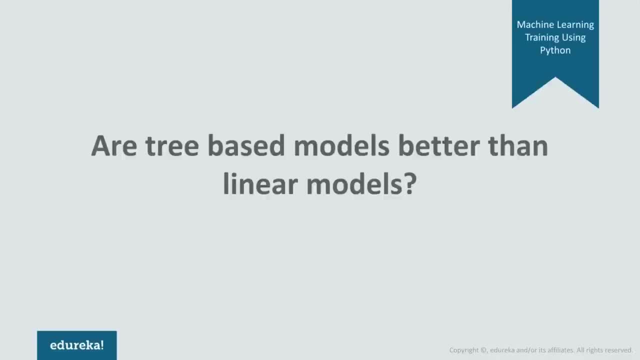 Let's look at some key factor which will help you to decide which algorithm to use and when. so the first point being, if the relationship between dependent and independent variable is well approximated by a linear model, then linear regression will outperform tree based model. second case: 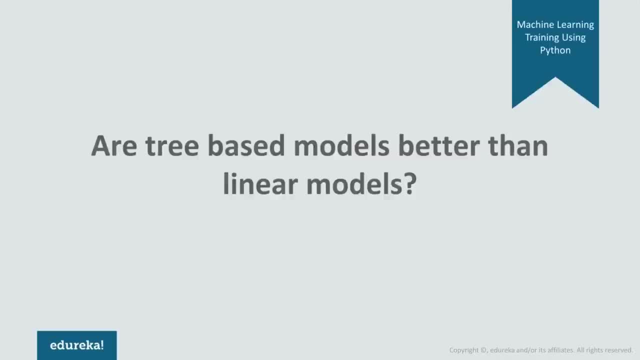 If there is a high non-linearity and complex relationship between dependent and independent variables, a tree model will outperform a classical regression model. In third case, if you need to build a model which is easy to explain to people, a decision tree model will always do better. 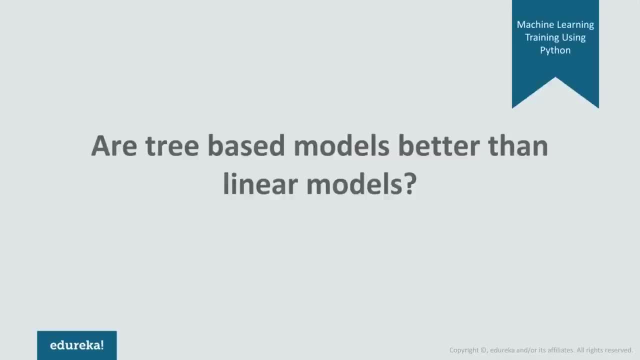 than a linear model, as the decision tree models are simpler to interpret than linear regression. All right, Now let's move on ahead and see how you can write a decision tree classifier from scratch and python using the cart algorithm. All right for this. 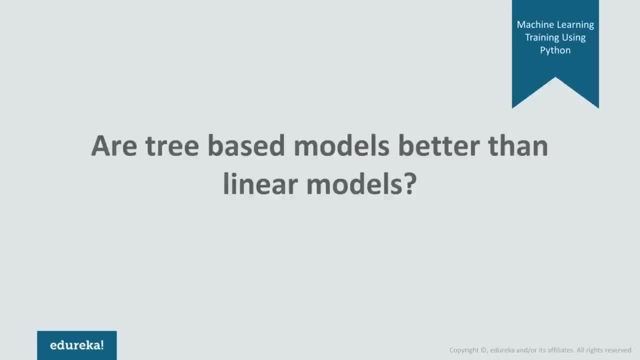 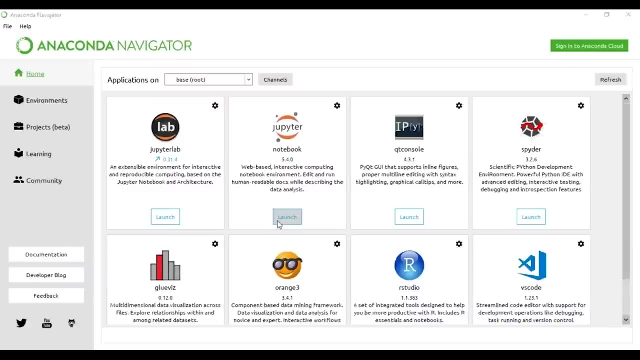 I'll be using Jupiter notebook with python 3.0 installed on it, All right, So let's open the Anaconda and the Jupiter notebook. Where is that? So this is our Anaconda Navigator, and I'll directly jump over to Jupiter notebook and hit the launch button. 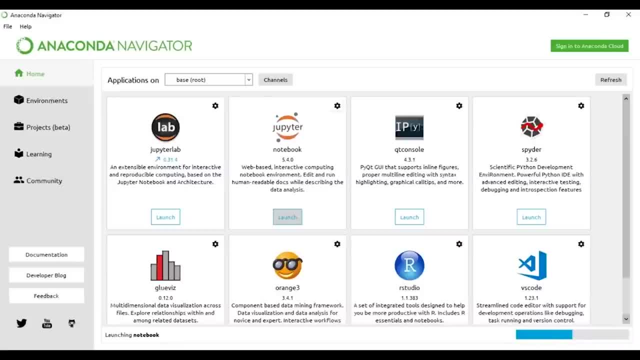 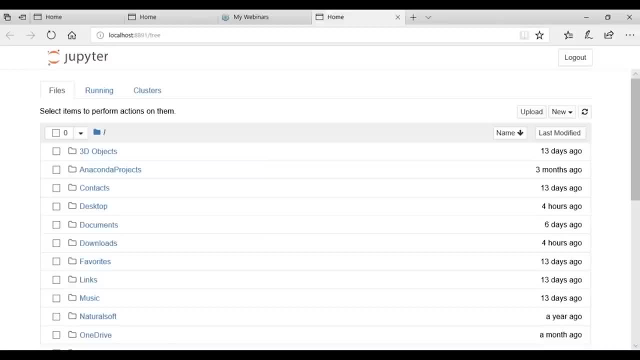 I guess everyone knows that Jupiter notebook is a web-based interactive computing notebook environment where you can run your python codes. So my Jupiter notebook- it opens on my localhost 8891.. So I'll be using this Jupiter notebook in order to write my decision tree classifier using python for this decision tree. 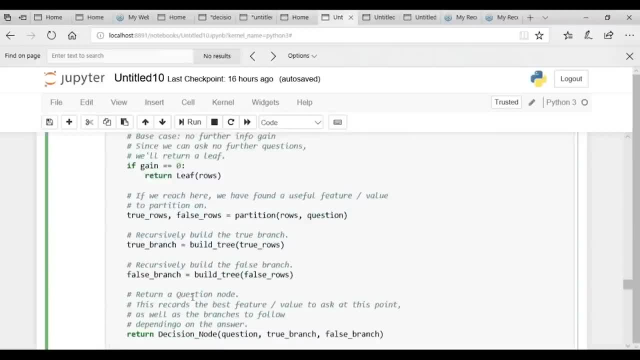 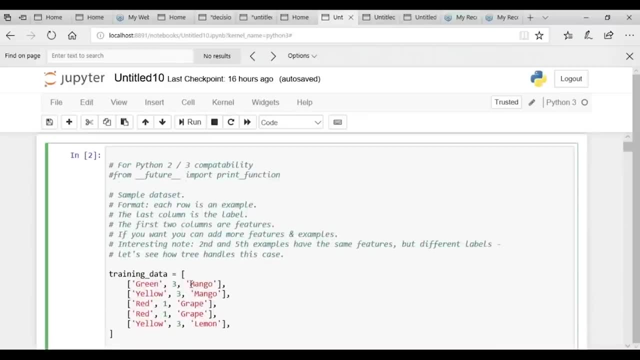 classifier. I have already written the set of codes. Let me explain you just one by one. So we'll start with initializing The training data set. So there's a sample data set for which each row is an example. The last column is a label and the first two columns are the. 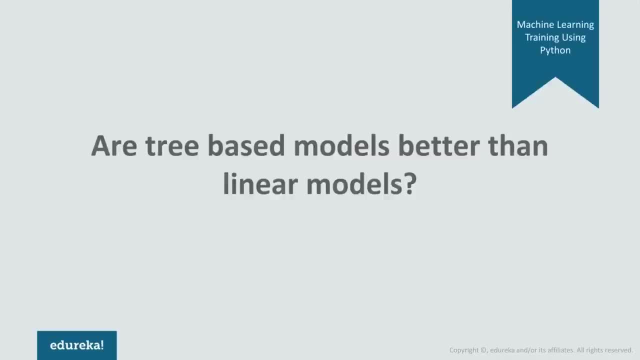 to explain to people. a decision tree model will always do better than a linear model, as the decision tree models are simpler to interpret than linear regression. All right, Now let's move on ahead and see how you can use the tree model, how you can write a decision tree classifier from scratch. 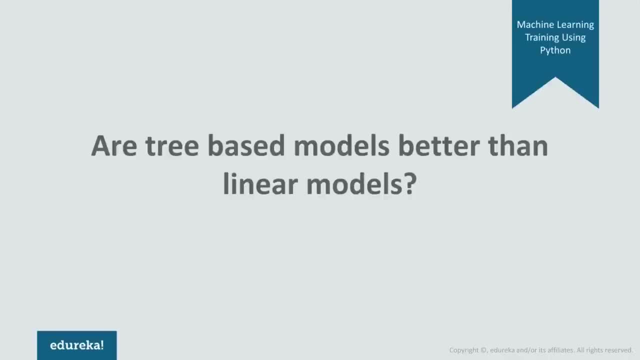 and python using the cart algorithm. All right, for this, I'll be using Jupiter notebook with python 3.0 installed on it. All right, So let's open the anaconda and the Jupiter notebook. Where is that? So there's a anaconda Navigator and I'll directly jump over. 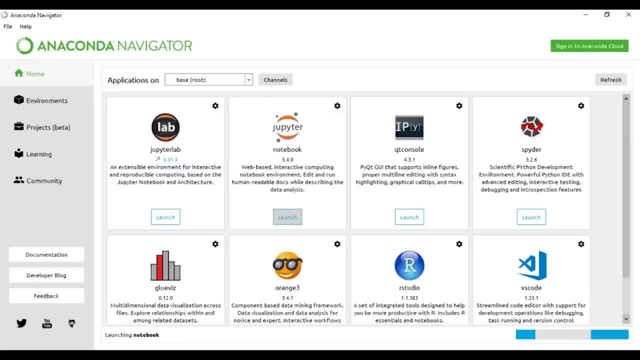 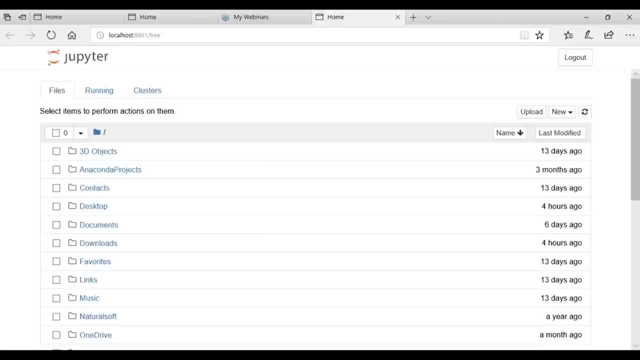 to Jupiter notebook and hit the launch button. I guess everyone knows that Jupiter notebook is a web-based interactive computing notebook environment where you can run your python codes. So my Jupiter notebook it opens on my localhost 8891. so I'll be using this Jupiter notebook in order to 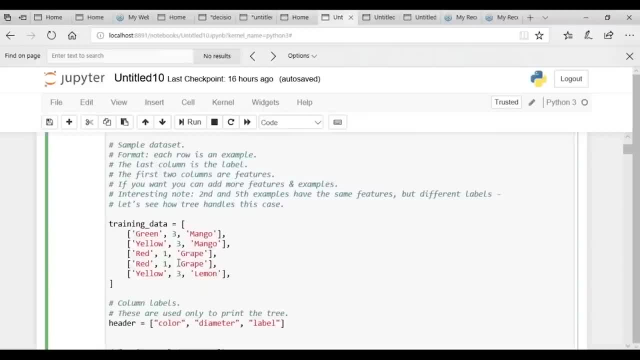 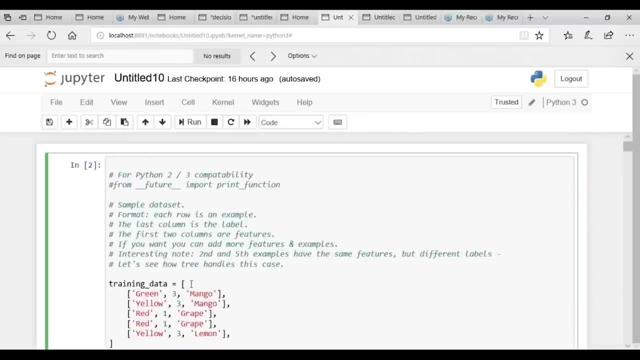 write my decision tree classifier using python. for this decision tree classifier, I have already written the set of codes. Let me explain you just one by one. So we'll start with initializing our training data set. So there's a sample data set for which each row is an example. 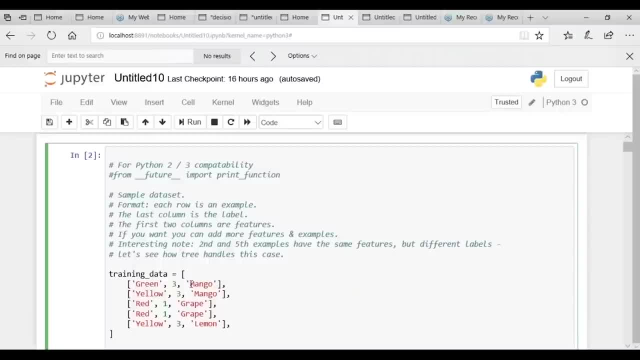 The last column is a label and the first two columns are the features. If you want, you can add some more features and example for your practice. Interesting fact is that this data set is designed in a way that the second and the fifth example have almost the same. 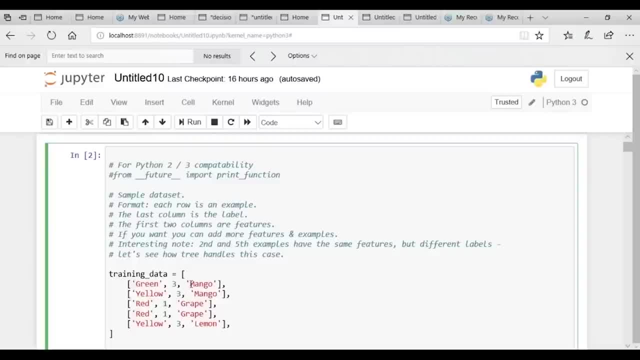 features, but they have different labels. All right, So let's move on and see how the tree handles this case. as you can see here, both of them- the second and the fifth column- have the same features. What they differ in is just their label. 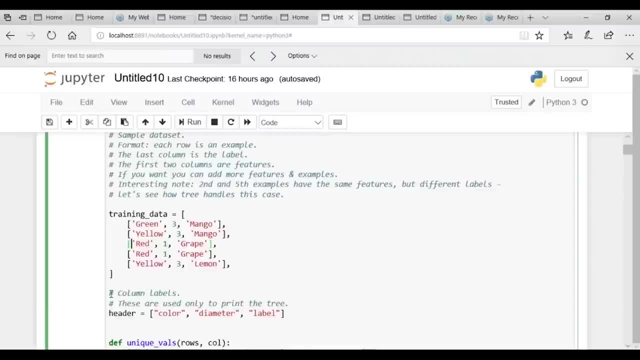 So let's move ahead. So this is our training data set. next, what we are doing: We are adding some column labels, So they are used only to print the trees. fine, So what we'll do? we'll add header to the columns, like the: 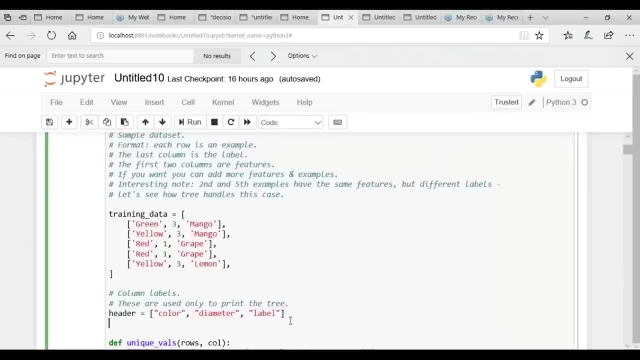 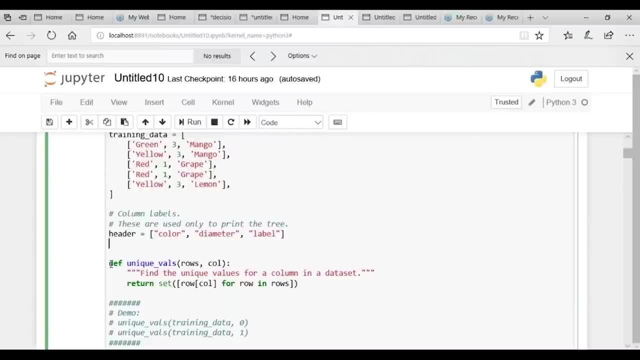 first column is of color, second is of diameter and third is of label column. All right, next, what we'll do will define a function as unique values, in which will pass the rows and the columns. So, this function, what it will do, it will find the unique values. 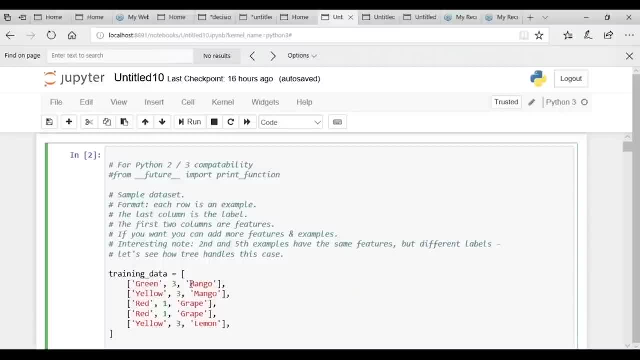 features. If you want, you can add some more features and example for your practice. Interesting fact is that this data set is designed in a way that the second and the fifth example have almost the same features, but they have different labels. All right, so let's move on and see how the tree handles this. 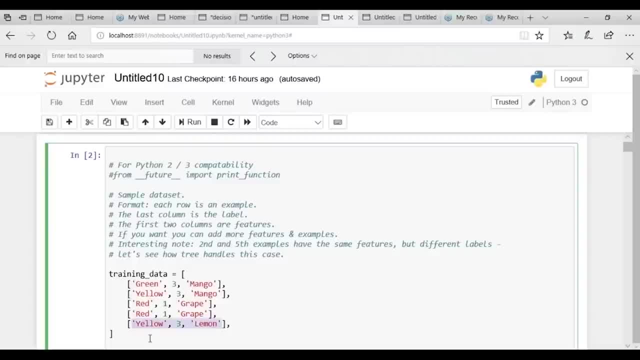 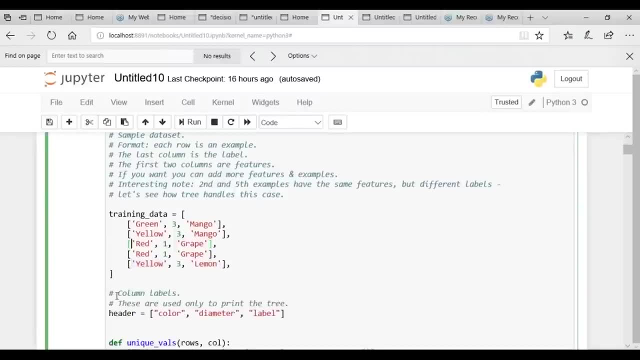 case. As you can see here, both of them- the second and the fifth column- have the same features. what they differ in is just their label. So let's move ahead. So there's our training data set. next, what we are doing, We are adding some column labels. 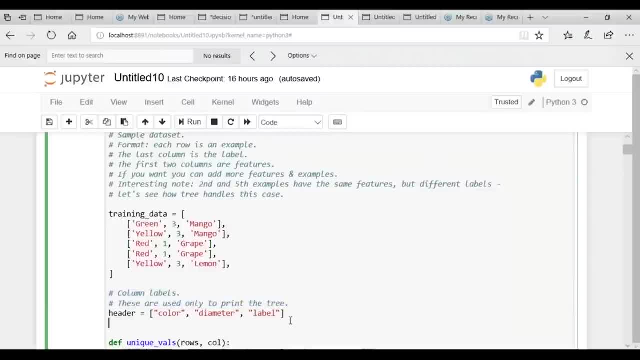 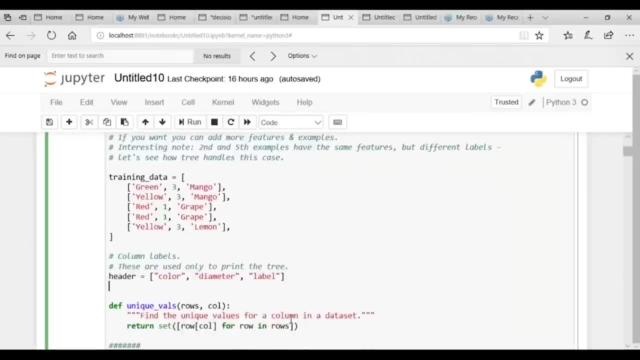 So they are used only to print the trees. fine, So what we'll do will add header to the columns, like the first column is of color, second is of diameter and third is of label column. All right. next, what we'll do will define a function as unique. 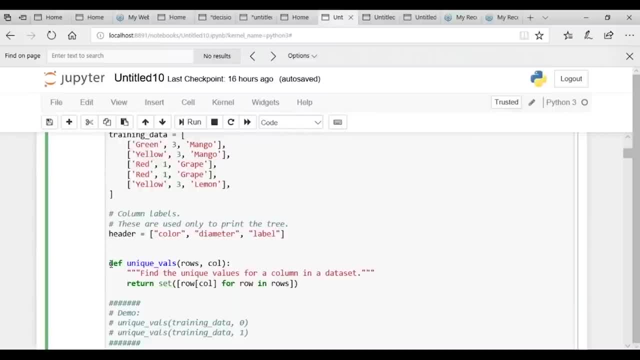 values in which will pass the rows and the columns. So this function, what it will do: it will find the unique values for a column in the data set. So there's an example for that. So what we are doing here, We are passing training data as our own and column number as 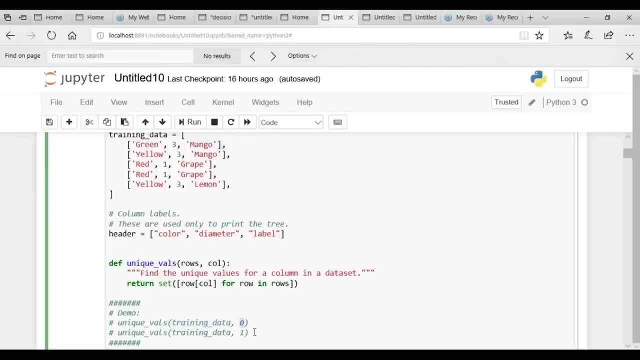 zero. So what we are doing, we are finding unique values in terms of color and in this, since the row is training data and the column is one, So what you are doing here. So we are finding the unique values in terms of diameter, fine. 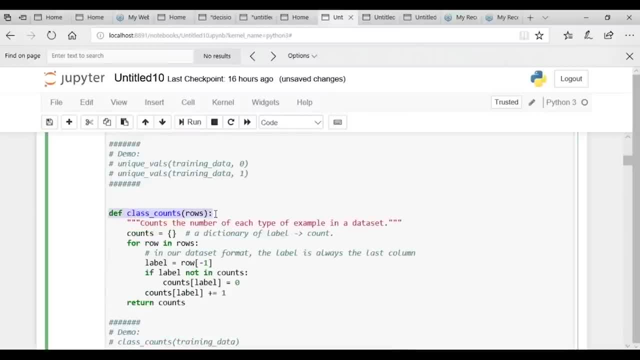 So this is just an example. next, what we'll do will define a function as class count and will pass the rows into it. So what it does, it counts the number of each type of example with an data set. So in this function, what we are basically doing? we are counting. 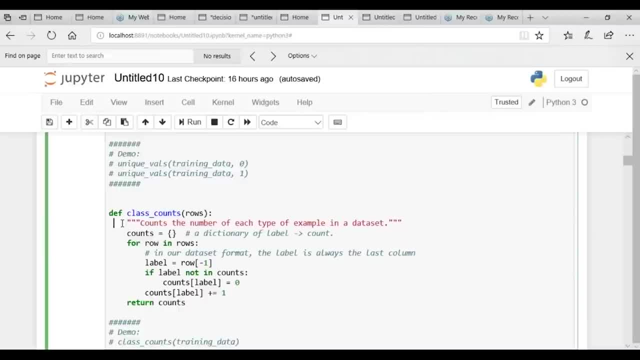 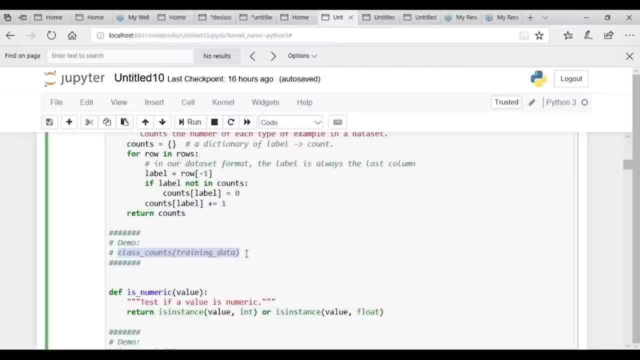 the number of each type, for example in the data set or what we are doing. We are counting the unique values for the label in the data set. as a sample You can see here We can pass that entire training data set to this particular function as class underscore count what it will do. 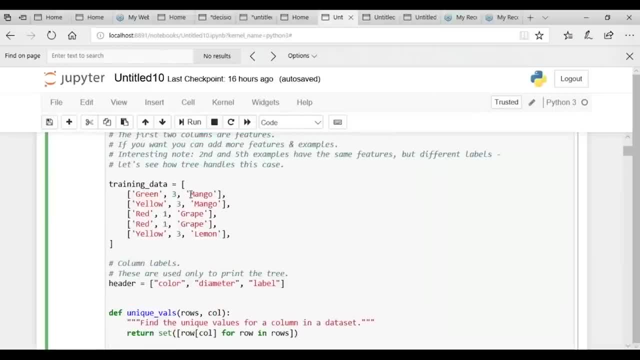 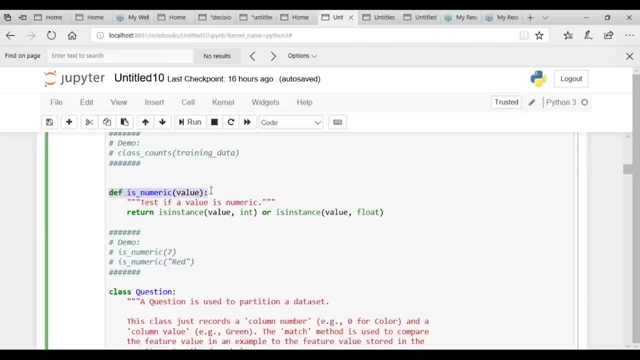 It will find all the different types of label within the training data set. as you can see here, the unique label consists of mango, grape and lemon. So next, what we'll do will define a function is numeric and will pass our value into it. So what it will do, it will just test if the value is numeric. 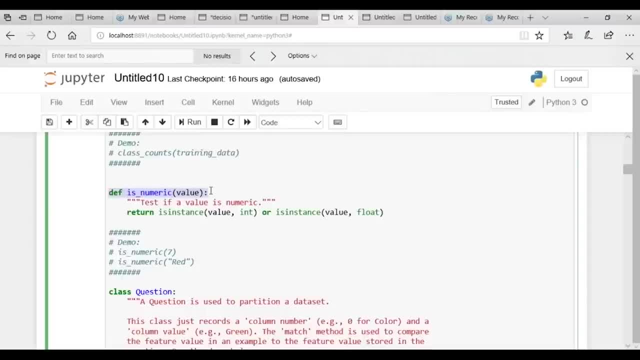 or not, and it will return. If the values and integer or a float, for example, you can see, is numeric. We are passing seven, So it has an integer, So it will return an int value and if you are passing red, it's not a numeric value. 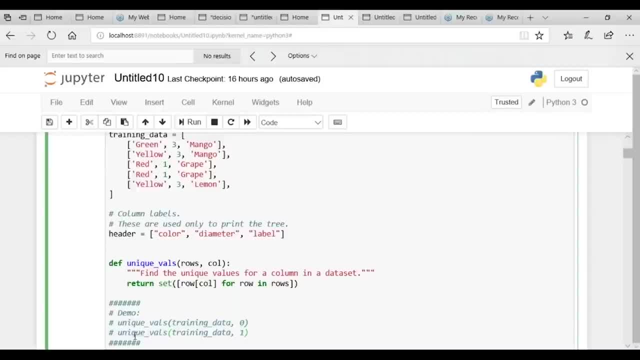 for a column in the data set. So there's an example for that. So what we are doing here, we are passing training data as our row and column number as zero. So what we are doing, we are finding unique values in terms of color and in this, since the row is training data and the 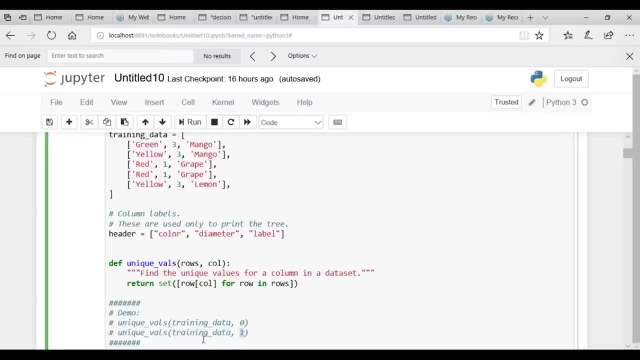 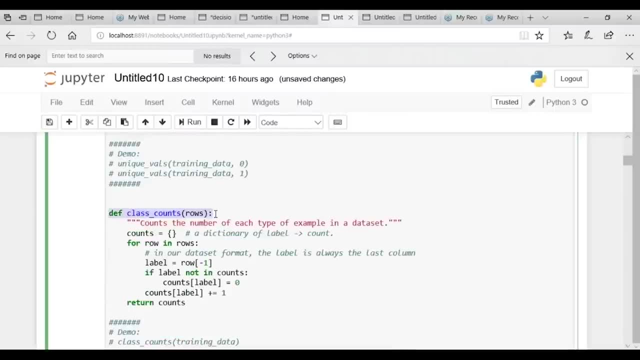 column is one. So what you are doing here? So we are finding the unique values in terms of diameter, Fine, So this is just an example. next, what we'll do will define a function as class count and will pass the rows into it. 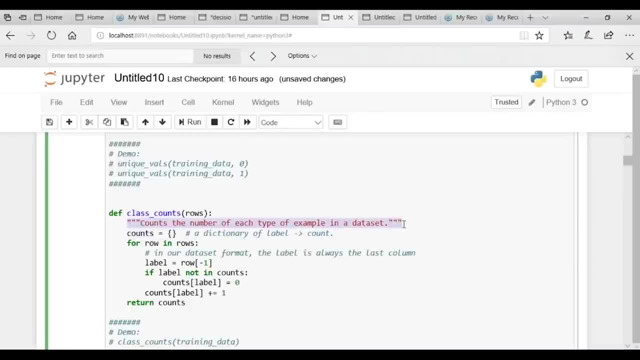 So what it does, it counts the number of each type of example with an data set. So in this function, what we are basically doing, we are counting the number of each type, for example, in the data set. or what we are doing We are counting the unique values for the label in the data. 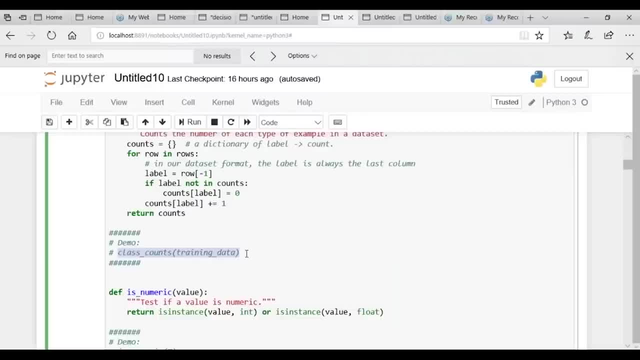 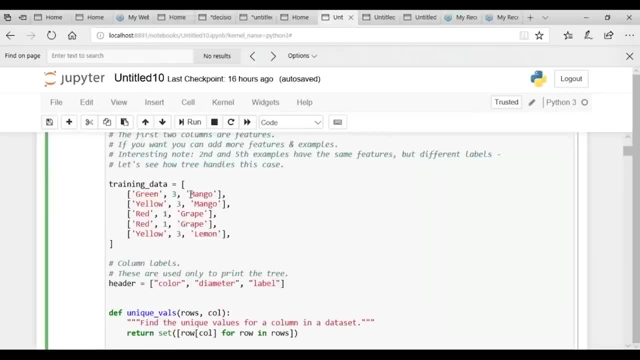 set as a sample. You can see here. We can pass that entire training data set to this particular function as class underscore count. what it will do? It will find all the different types of label within the training data set. As you can see here, the unique label consists of mango grape. 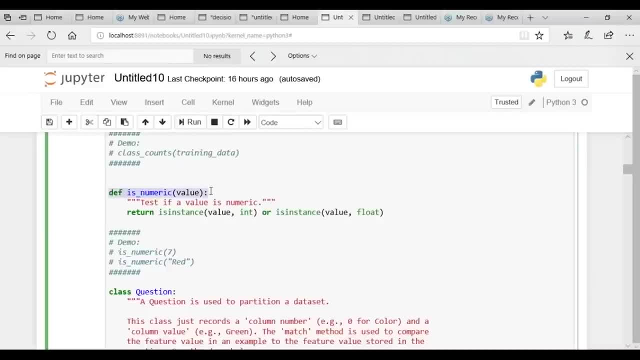 and lemon. So next, what we'll do will define a function is numeric and will pass a value into it. So what it will do, it will just test if the value is numeric or not and it will return if the values and integer or a float. 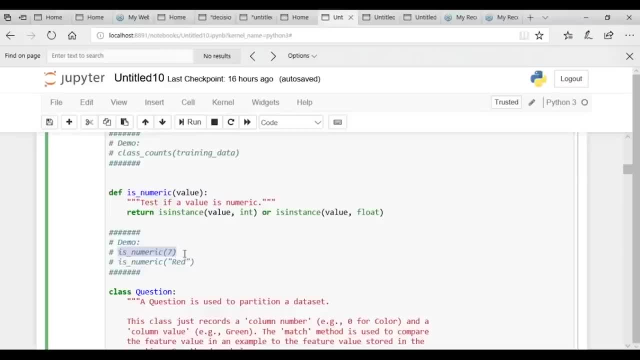 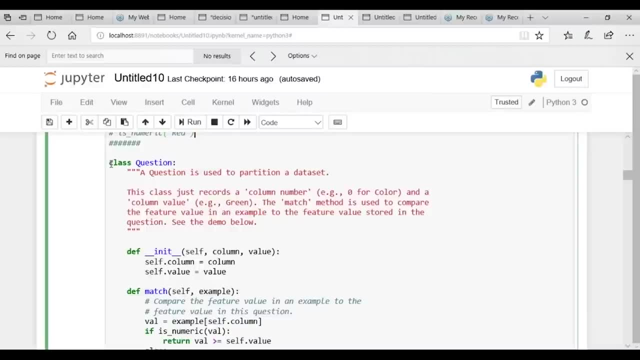 for example you can see, is numeric. We are passing seven, So it has an integer, So it will return an int value, and if you are passing red, it's not a numeric value, right? So moving on ahead will define a class named as question. 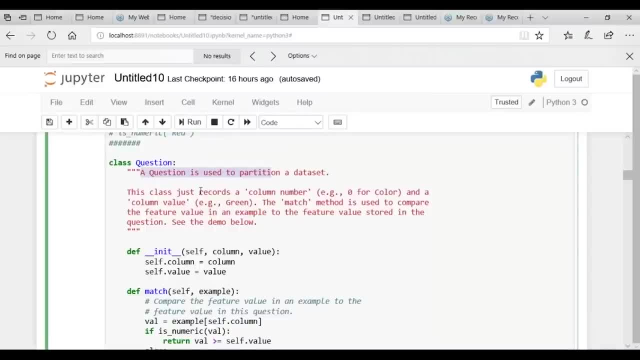 So what this question does? this question Is used to partition the data set, this class. what it does? It just records a column number, For example 0 for color light, and a column value, For example green. next, what we are doing? We are defining a match method which is used to compare the 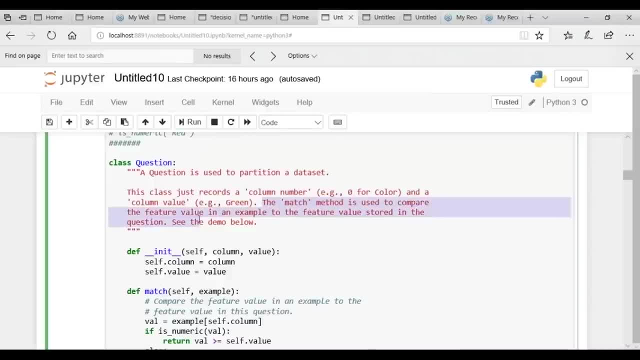 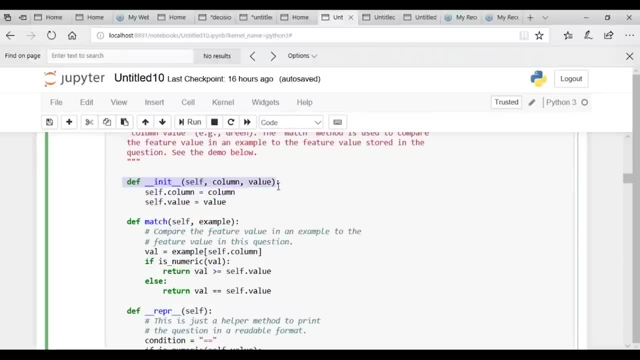 feature value in the example to the feature value stored in the question. Let's see how. first of all, what we are doing. We're defining an init function and inside that we are passing the self column and the value as parameter. So next, what we do. we define a function as match what it does. 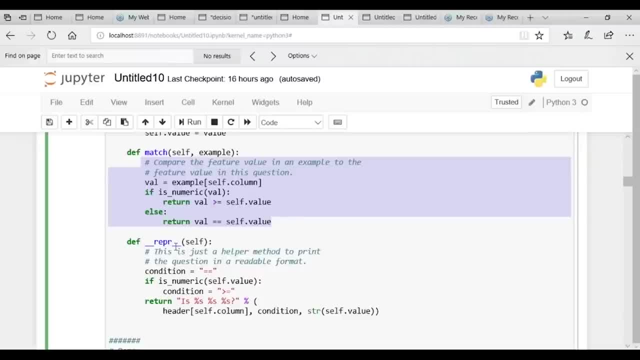 it compares the feature value And an example to the feature value in this question, when next will define a function as our EPR, which is just a helper method to print the question in a readable format. next, what we are doing: We are defining a function, partition. 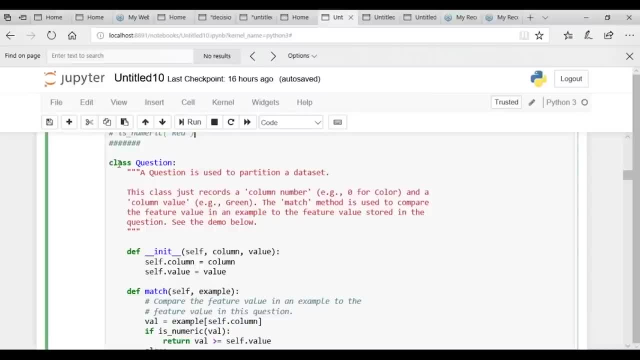 right, So moving on ahead, will define a class named as question. So what this question does? this question is used to partition the data set this class, what it does? it just records a column number, for example 0 for color, a light, and a column value. 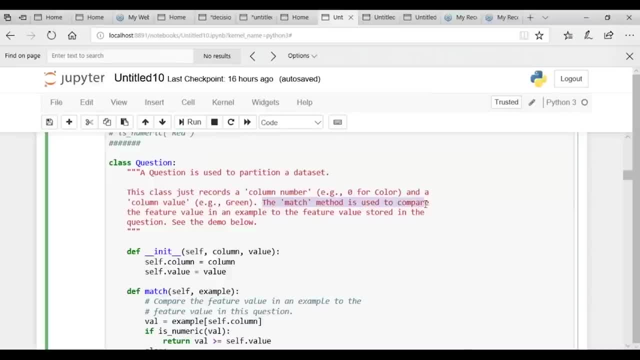 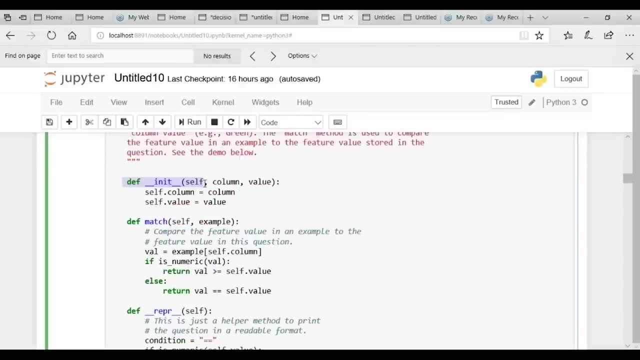 for example, green. next, what we are doing: we are defining a match method which is used to compare the feature value in the example to the feature value stored in the question. Let's see how. first of all, what we are doing: We're defining an init function and inside that we are passing. 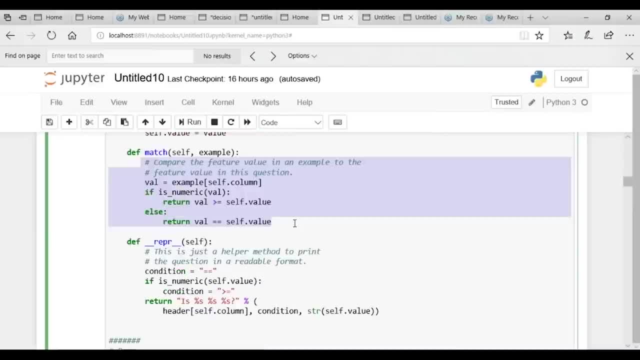 the self column and the value as parameter. So next, what we do? we define a function as match what it does. it compares the feature value in an example to the feature value in this question. Fine, next will define a function as our EPR, which is just: 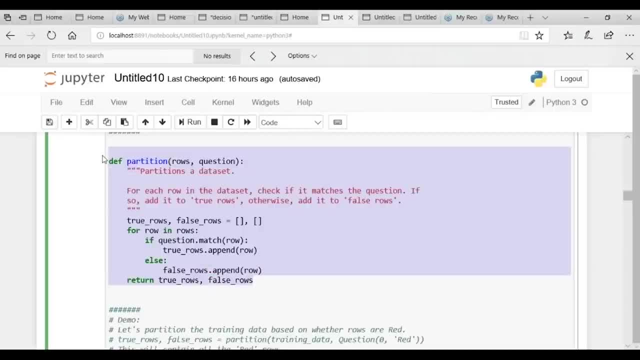 a helper method to print the question in a readable format. Next, what we are doing? We are defining a function: partition. Well, this function is used to partition the data set. each row in the data set. it checks if it matches the question or not. if it does so, it adds it to the true rows, or if not, then 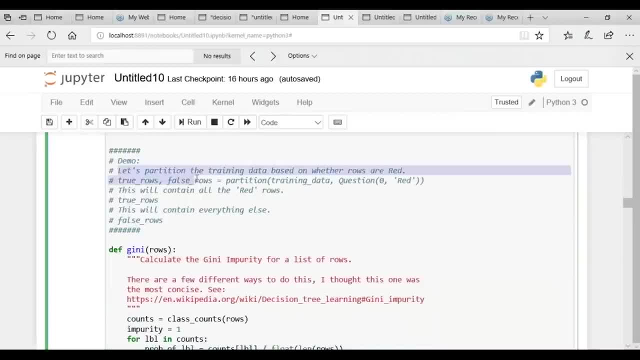 it adds to the false rows. All right, for example, as you can see here, let's partition the training data set based on whether the rows are red or not. here We are calling the function question and we are passing a value of 0 and red to it. 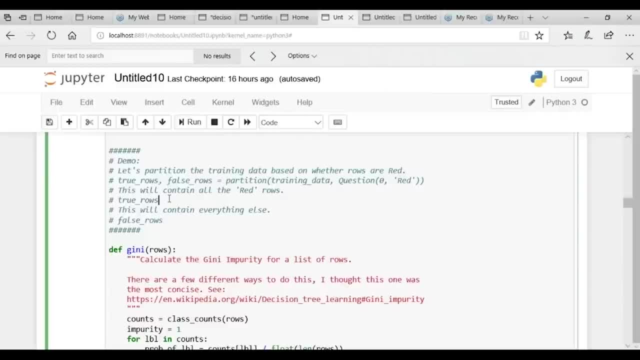 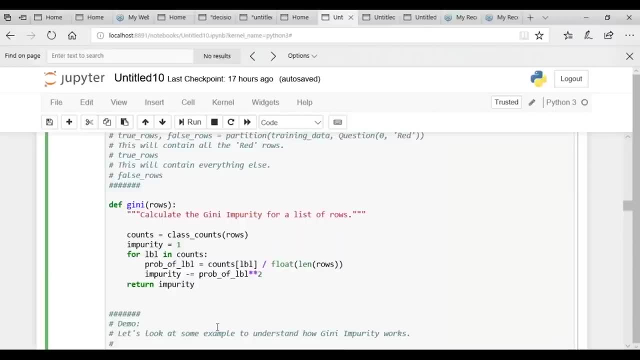 So what it will do, it will assign all the red Rose to true underscore Rose and everything else will be assigned to false underscore Rose. Fine, next, what we'll do will define a genie impurity function and inside that will pass the list of rows. So what it will do, it will just calculate the genie impurity. 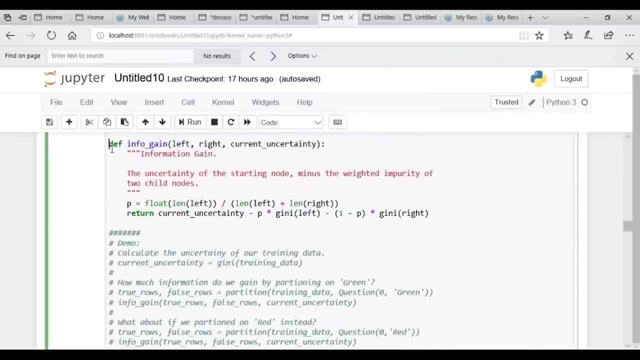 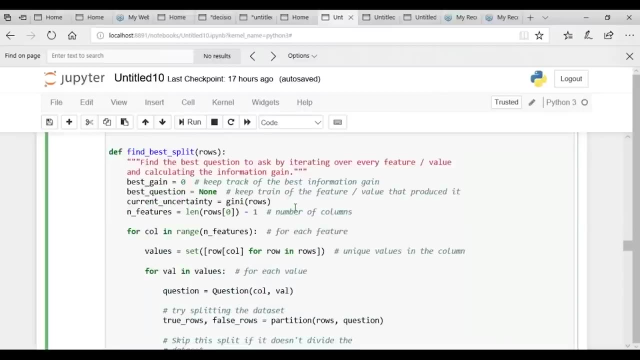 for the list of rows. Next, what we are doing here with defining a function as information gain. So what this information gain function does? it calculates the information gain using the uncertainty of the starting node minus the weighted impurity of the child known. the next function is find the best split. 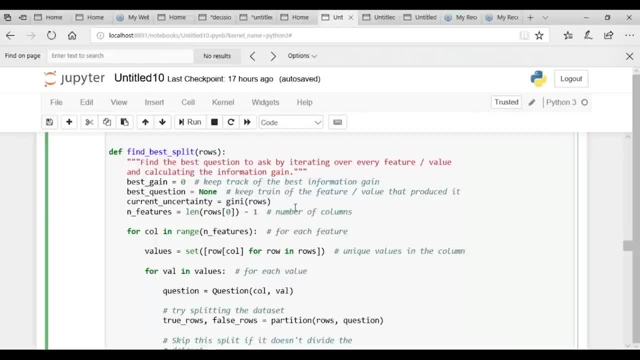 Well, this function is used to find the best question to ask by iterating over every feature or value and then calculating the information gain. For the detail explanation on the code, You can find the code in the description given below. All right, next we'll define a class as leave for classifying. 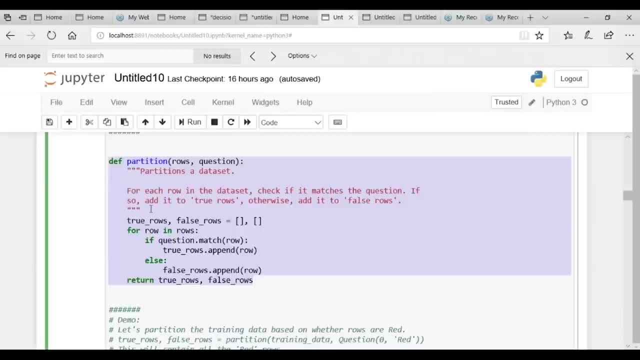 Well, this function is used to partition the data set. each row in the data set, It checks if it matches the question or not. if it does so, it adds it to the true rows, or if not, then it adds to the false rows. All right, for example, as you can see here, let's partition. 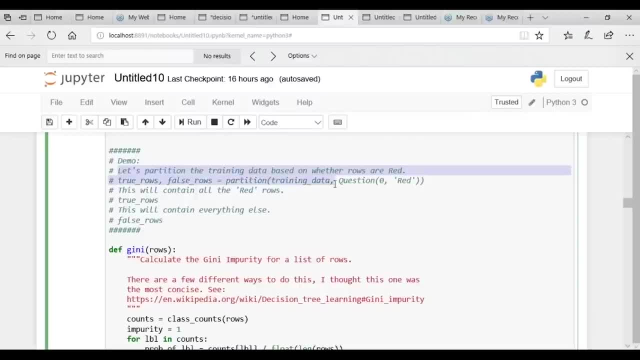 the training data set based on whether the rows Are red or not. here We are calling the function question and we are passing a value of 0 and red to it. So what it will do? it will assign all the red rose to true underscore Rose and everything else will be assigned to false. 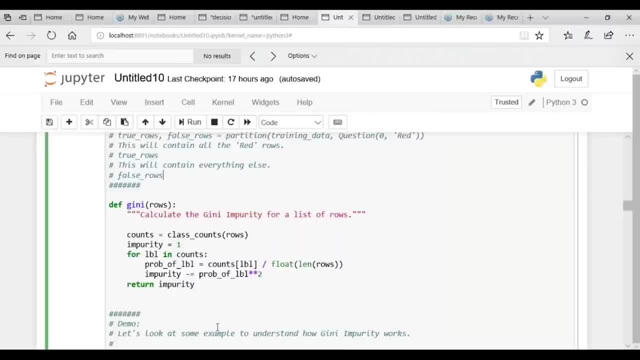 underscore Rose, fine. Next, what we'll do will define a genuine purity function and inside that will pass the list of Rose. So what it will do, it will just calculate the gene impurity for the list of Rose. Next, what we are doing here with defining a function as 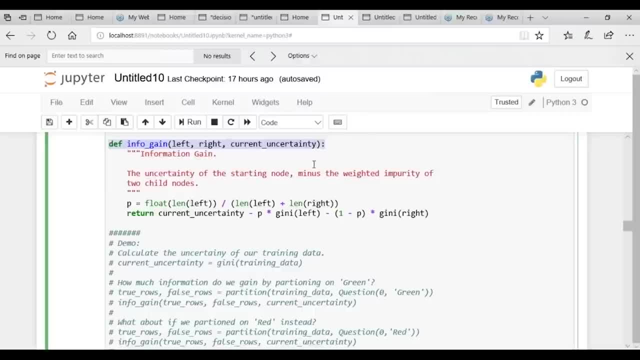 information gain. So what does information gain Function does? it calculates the information gain using the uncertainty of the starting node minus the weighted impurity of the child node. The next function is find the best split. Well, this function is used to find the best question to ask. 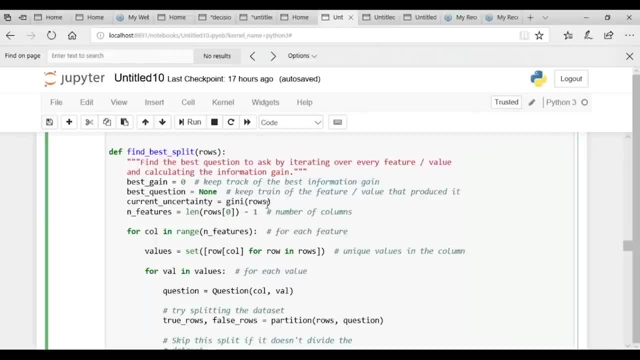 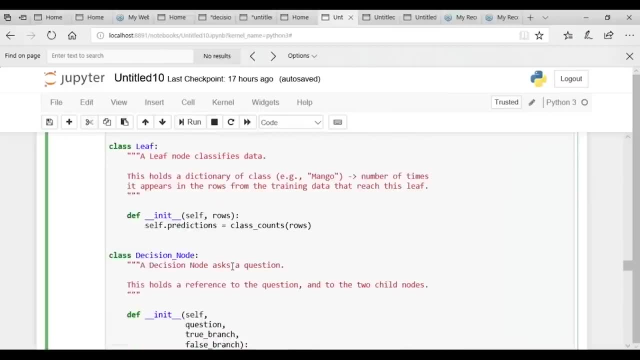 by iterating over every feature or value and then calculating the information gain. for the detail explanation on the code, You can find the code in the description given below. All right. Next we'll define a class as leaf for classifying the data It holds, a dictionary of class like mango for. 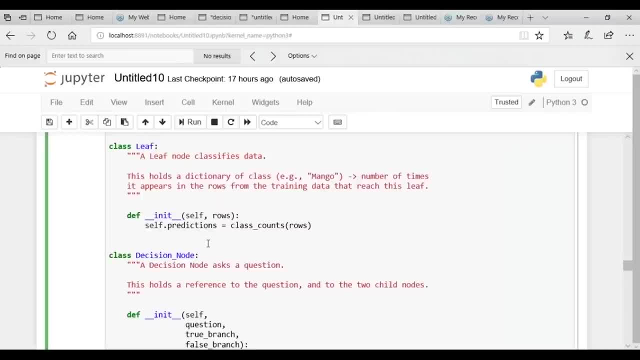 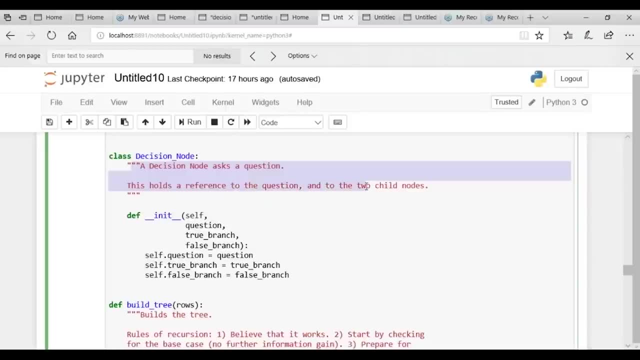 How many times it appears in the row from the training data. that reaches the sleeve. All right, Next is the decision node. So this decision node, it will ask a question. This holds a reference to the question and the two child nodes on the base of it. 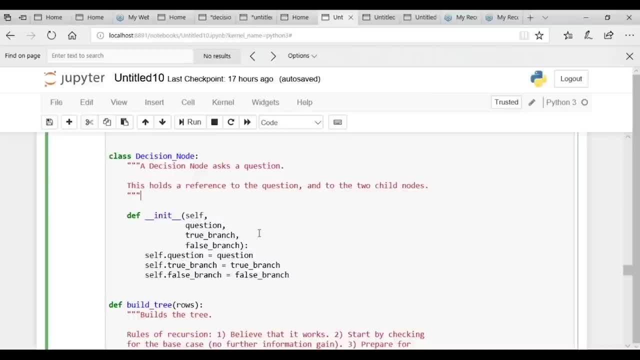 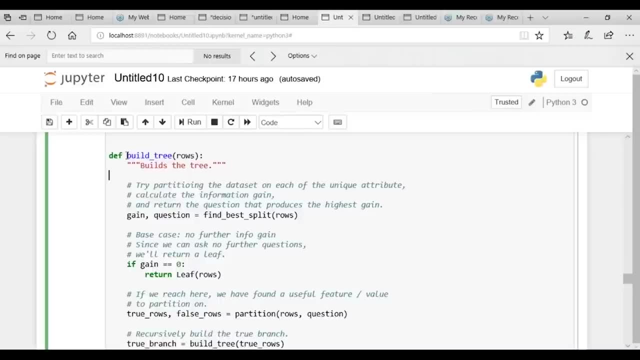 You are deciding which node to add further to which branch. All right, So next, what we are doing, we are defining a function of build tree and inside that we are passing our number of rows. So this is the function that is used to build a tree. 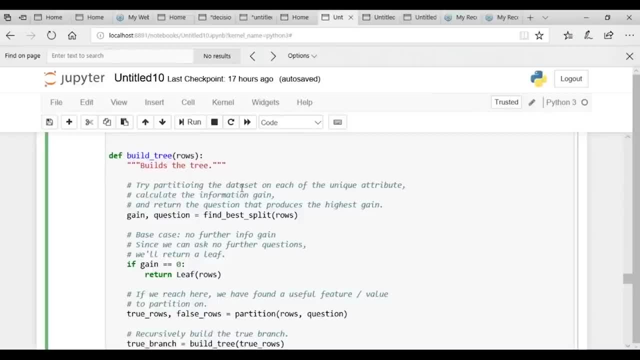 So, initially, what we did. we define all the various function that we will be using in order to build a tree. So let's start by partitioning the data set for each unique attribute, Then we'll calculate the information gain and then return the question that produces the highest gain, and on the basis. 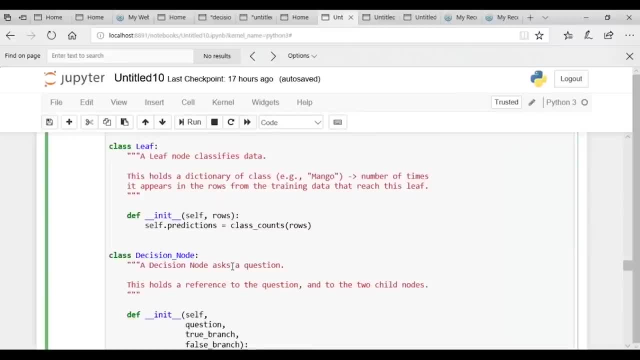 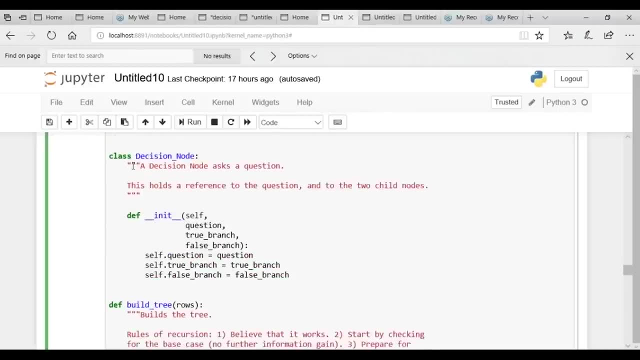 the data It holds. a dictionary of class like mango, for how many times it appears in the row from the training data that reaches the sleeve. All right, next is the decision node. So this decision node, it will ask a question. This holds a reference to the question and the two child nodes. 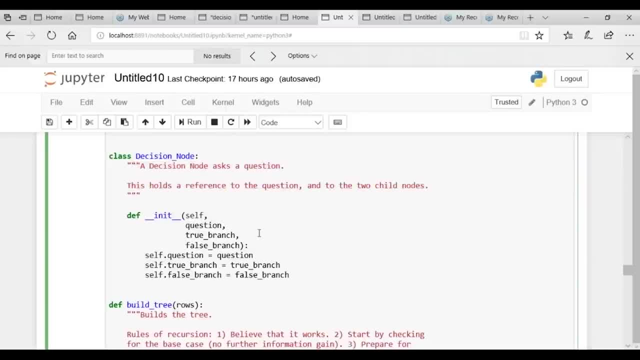 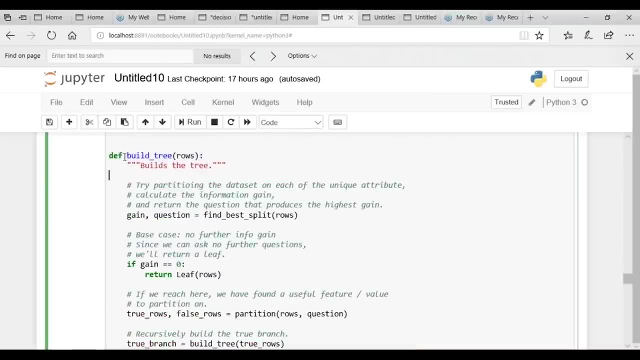 On the basis of it, You are deciding which node to add further to which branch. All right, So next, what we are doing? we are defining a function of build tree and inside that we are passing our number of rows. So this is the function that is used to build a tree. 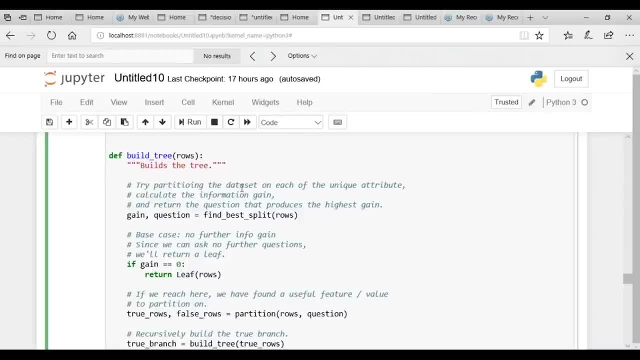 So, initially, what we did. we define all the various function that we will be using in order to build a tree. So let's start by partitioning the data set for each unique attribute, then will calculate the information gain and then return the question that produces the highest game. and on, 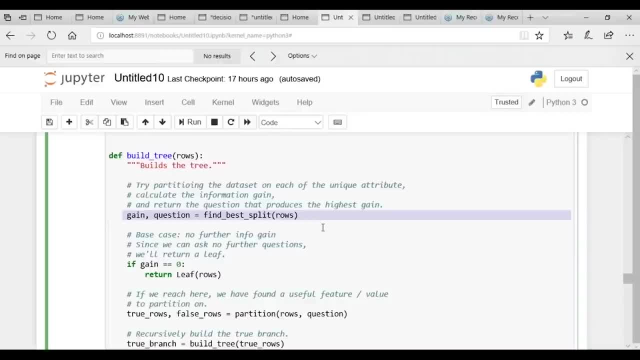 the basis of that, We'll split the tree. So what we are doing here, We are partitioning the data set, calculating the information gain and then what this is returning. It is returning the question that is, producing the highest game. All right. 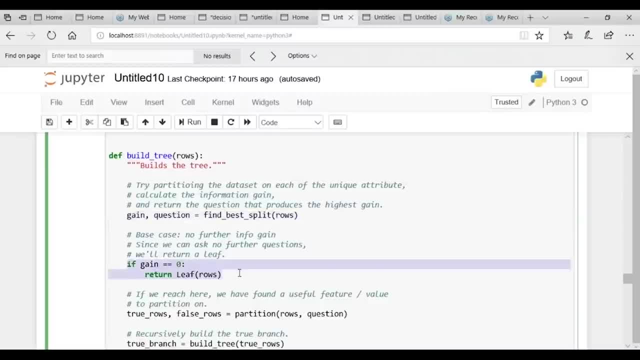 Now, if gain equals 0, return leaf arose. So what it will do? So if we are getting no for the gain, that is, gain equals 0, then in that case, since no further question could be asked, So what it will do? it will return a leaf. fine, now true. 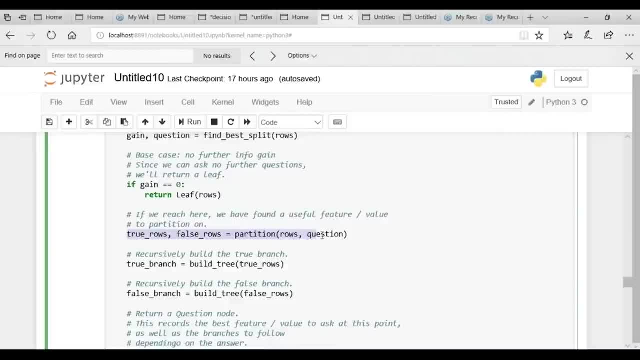 underscore rows of false underscore rows, Equal partition with rows and the question. So if we are reaching till this position, then you have already found a feature of value which will be used to partition the data set. then what you will do? you will recursively build the. 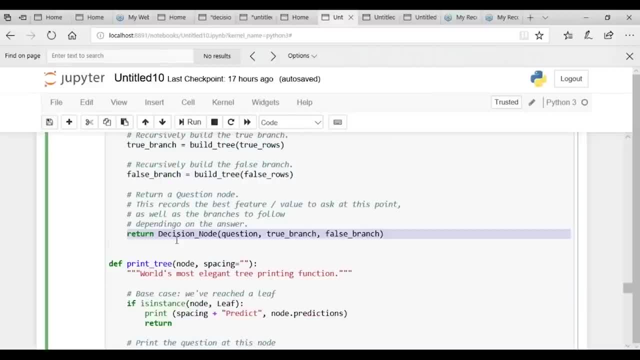 true branch and similarly recursively build the false branch. So return decision underscore node and inside that will be passing question: true branch and false branch. So what it will do, it will return a question node and this question node. this records the best feature or the value to 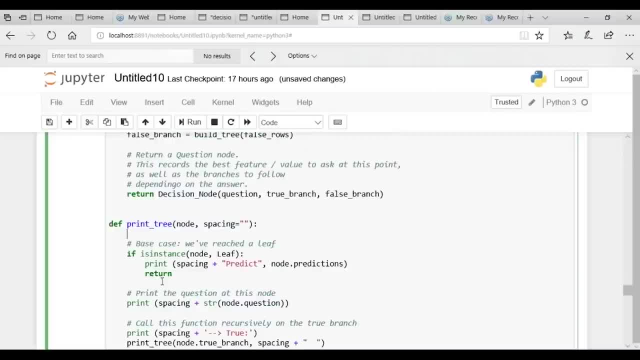 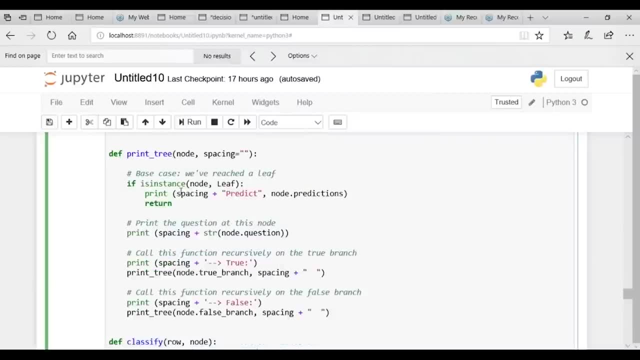 ask at this point: fine, now that we have built our tree. Next, what we'll do will define a print underscore tree function which will be used to print the tree. fine, So, finally, what we are doing in this particular function that we are printing our tree. next is the classify function, which 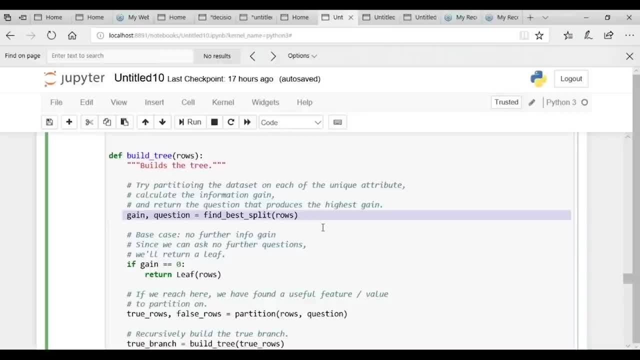 of that will split the tree. So what we are doing here? we are partitioning the data set, calculating the information gain, and then what this is returning. It is returning the question that is, producing the highest gain. All right Now, if gain equals 0, return leaf rows. so what it will do. 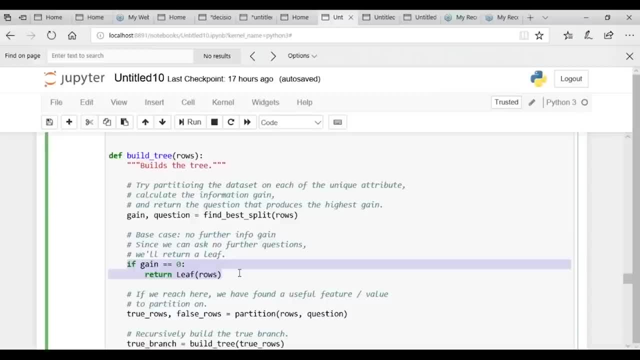 So if you are getting no for the gain- that is, gain equals 0- then in that case, since no further question could be asked, So what it will do, it will return a leaf. fine, Now, true underscore rows of false underscore rows, equal partition with rows and the question. 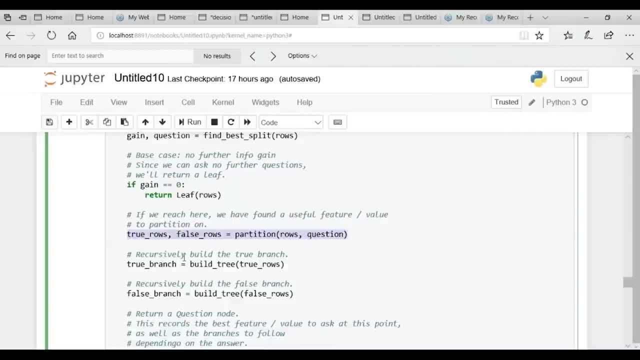 So if we are reaching till this position, then you have already found a feature of value which will be used to partition the data set. Then what you will do? you will recursively build the true branch and similarly recursively build the false branch. So return decision underscore. 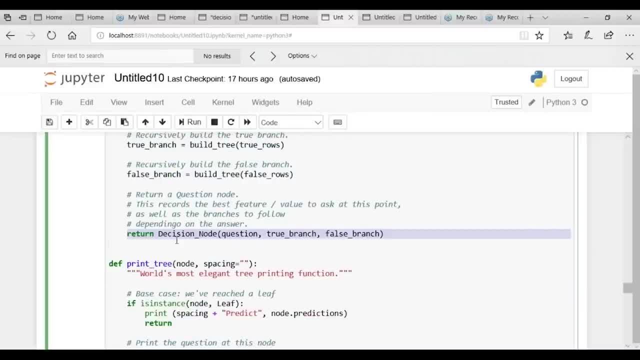 node and inside that will be passing question to branch and false branch. So what it will do, it will return a question node and this question node. This records the best feature or the value to ask at this point. Fine, Now that we have build our tree. next, what we'll do will: 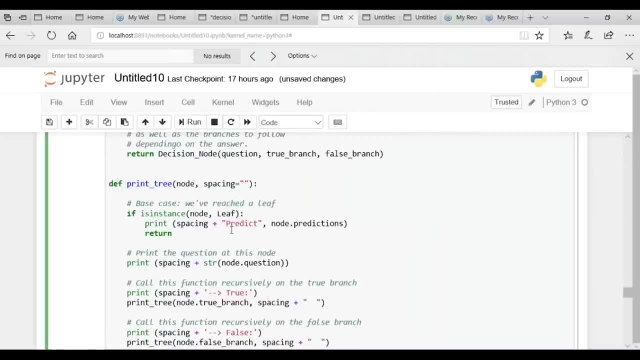 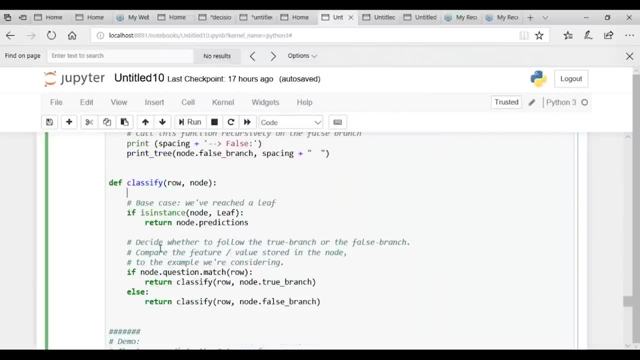 define a print underscore tree function which will be used to print the tree. fine, So, finally, what we are doing in this particular function, that we are printing our tree. Next is the classify function, which will use it to decide whether to follow the true branch or the false branch, and 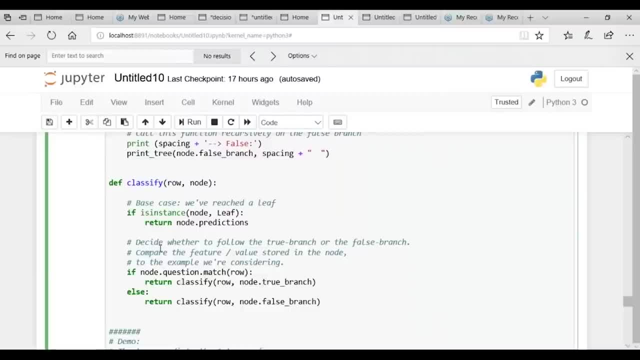 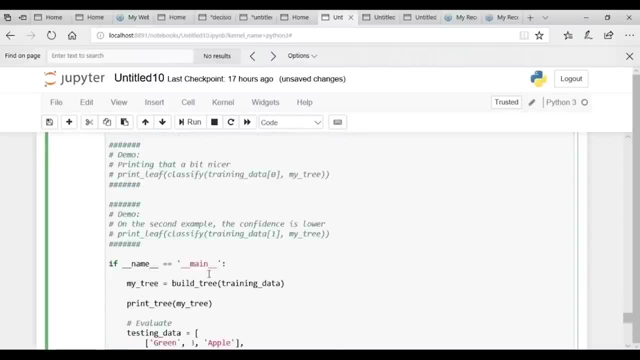 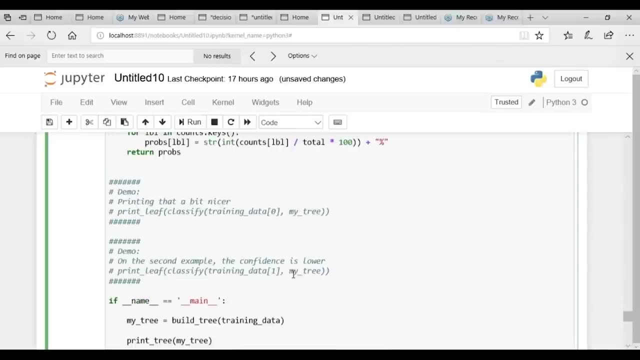 then compare to the feature of values stored in the node, to the example we are considering, and, last, what we'll do will finally print the prediction and leave, So let's execute it and see: Okay, So there's our testing data. All right, so we printed our leaf as well. 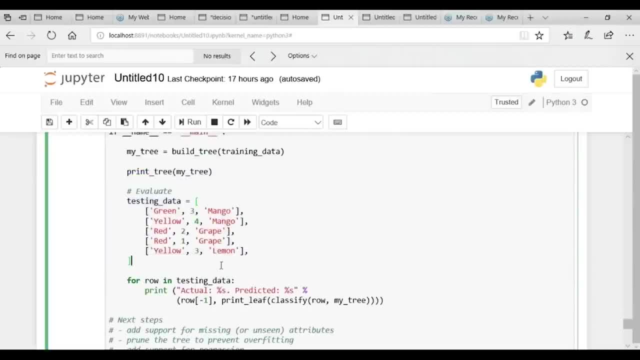 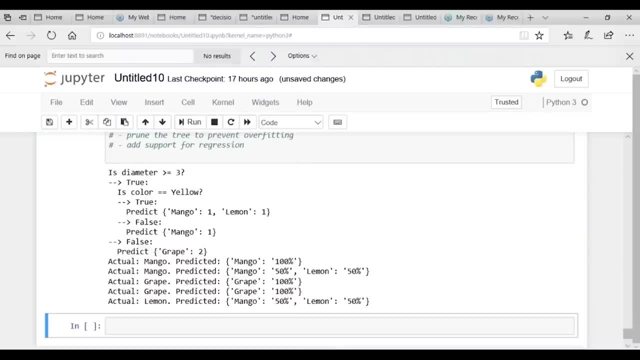 Now that we have trained our algorithm with our training data set, now it's time to test it. So there's our testing data set, So let's finally execute it and see what is the result. So this is the result you will get. 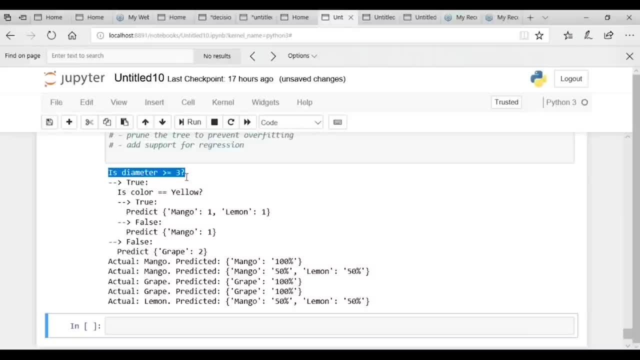 So first question which is asked by the algorithm is: is diameter greater than equal to 3? if it is true, then it will further ask if the color is yellow. again, if it is true, then it will predict mango as one and lemon with one. 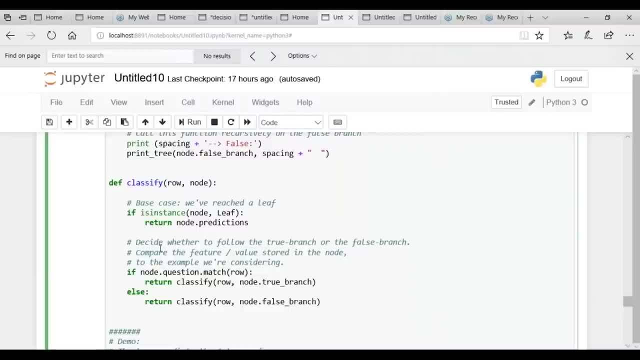 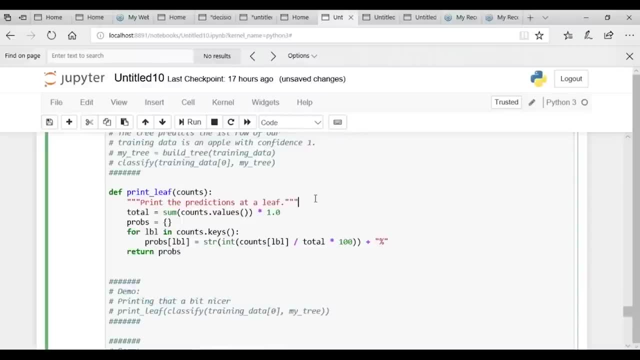 will use it to decide whether to follow the true branch or the false branch, and then compare to the feature of values stored in the node, to the example We are considering. and last, what we'll do will finally print the production and leave. So let's execute it and see. 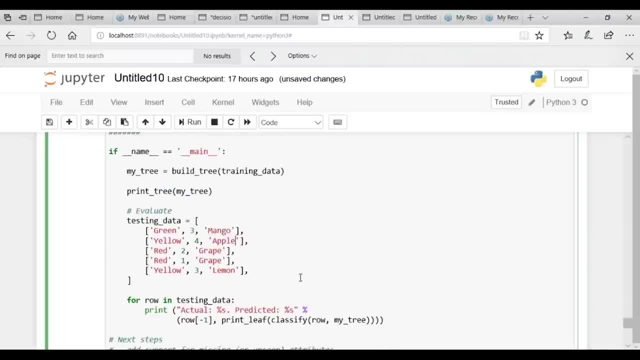 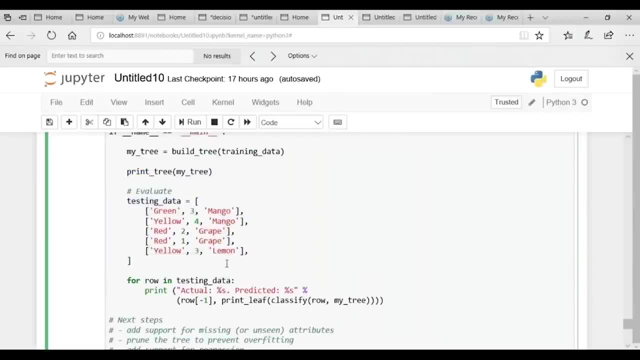 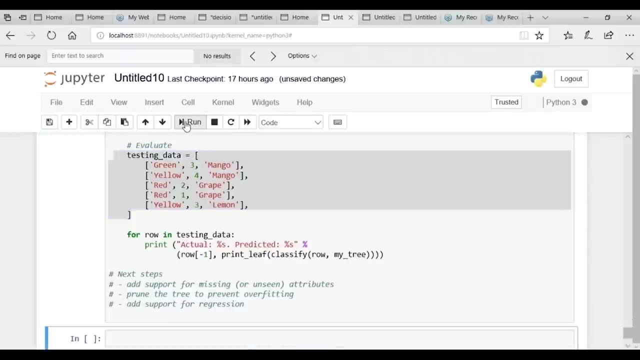 Okay, So there's our testing data. All right, so we printed our leaf as well. Now that we have trained our algorithm with our training data set, now it's time to test it. So there's our testing data set. So let's finally execute it and see what is the result. 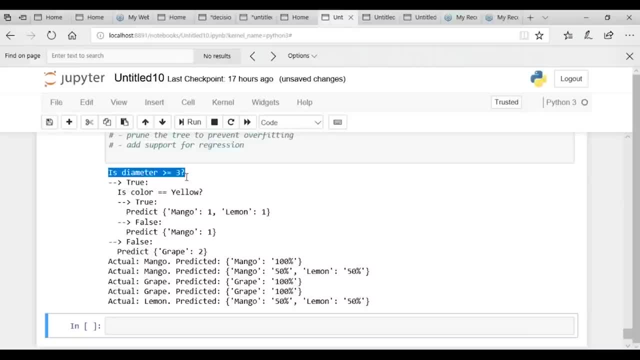 So this is the result you will get. So first question which is asked by the algorithm is: is diameter greater than equal to 3? if it is true, then it will further ask if the color is yellow. again, if it is true, then it. 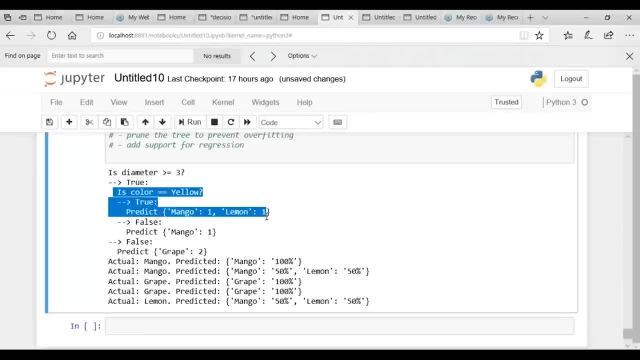 will predict mango as one And lemon with one, All right. and in case it is false, then it will just predict the mango. Now, this was the true part. Now, next coming to, diameter is not greater than or equal to 3.. 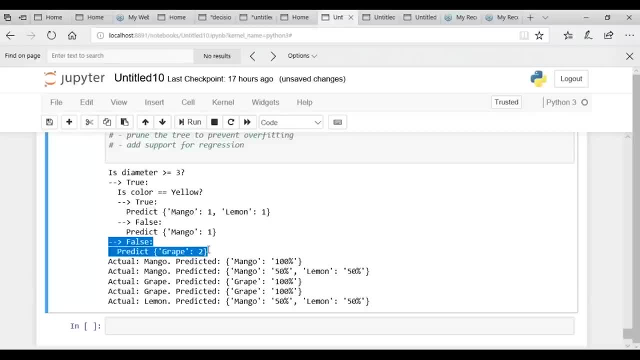 Then in that case it's false. and what it will do? It will just predict the grape. fine, Okay, So this was all about the coding part. Now let's conclude this session. But before concluding, let me just show you one more thing. 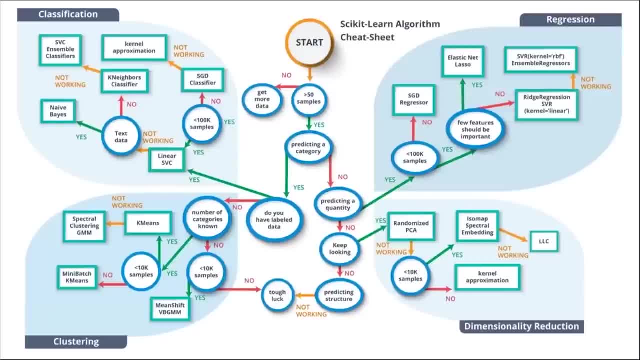 And there's a scikit-learn algorithm cheat sheet which explains you which algorithm you should use and when. All right, it's built in a decision tree format. Let's see how it is built. So, first condition: it will check whether you have 50 samples. 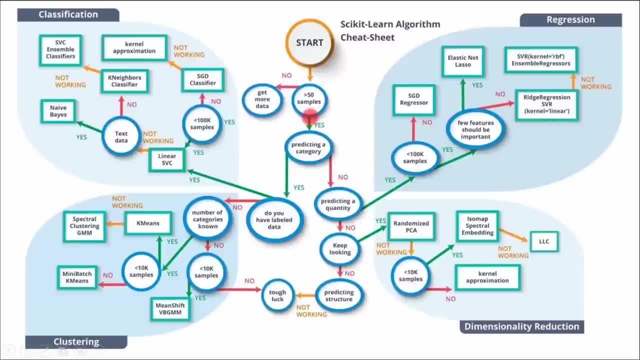 or not. If your samples are greater than 50, then it will move ahead. If it is less than 50, then you need to collect more data. If your sample is greater than 50, then you have to decide whether you want to predict a category or not. 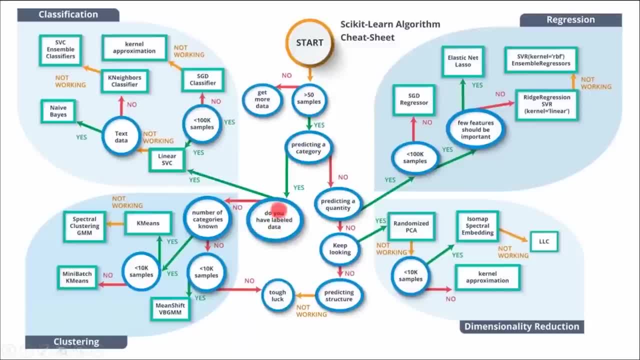 If you want to predict a category, then further you will see that whether you have label data or not, If you have label data, then that would be a classification algorithm problem. If you don't have the label data, then it would be a classification. 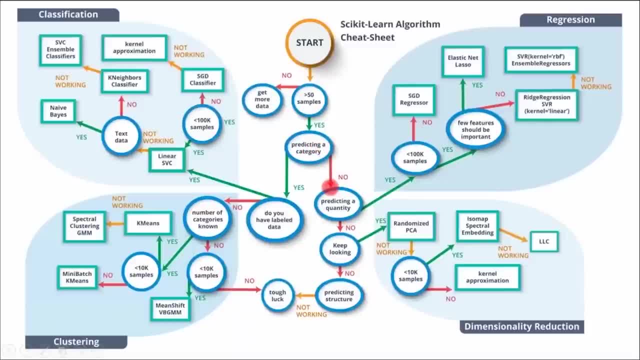 clustering problem. Now, if you don't want to predict a category, then what do you want to predict? Predict a quantity? Well, if you want to predict a quantity, then in that case it would be a regression problem. If you don't want to predict a quantity and you want to keep, 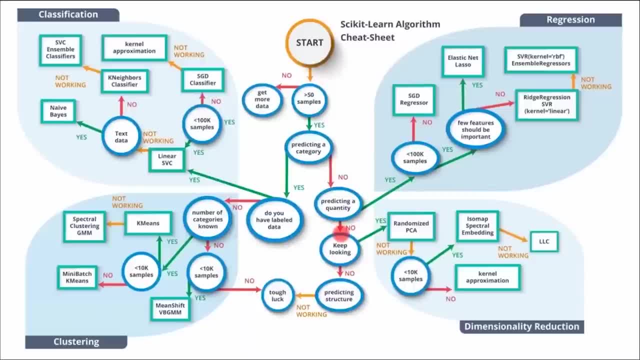 looking further, then in that case you should go for dimensionality reduction problems. And still, if you don't want to look and the predicting structures not working, then you have tough luck for that. I hope this decision tree session clarifies all your doubt. 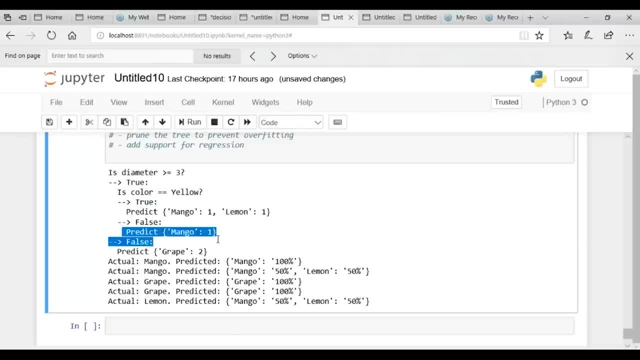 All right, and in case it is false, then it will just predict the mango. Now, this was the true part. Now, next, coming to, diameter is not greater than or equal to three, then in that case it's false and what it will do it. 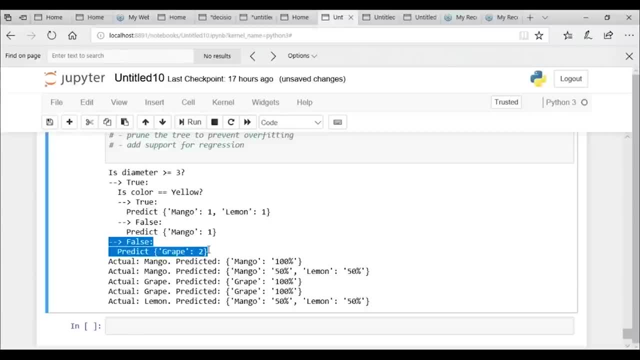 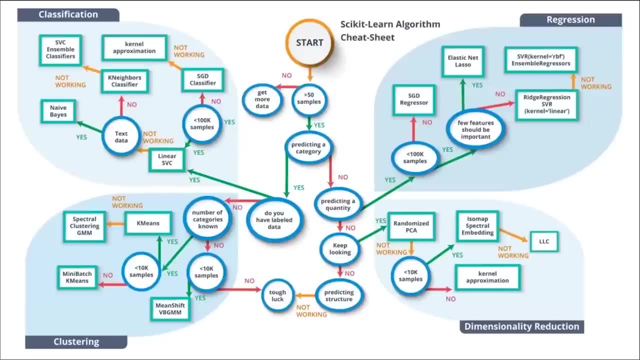 will just predict the grape, fine, Okay. So this was all about the coding part. Now let's conclude this session. But before concluding, let me just show you one more thing. Now there's a scikit-learn algorithm cheat sheet, which 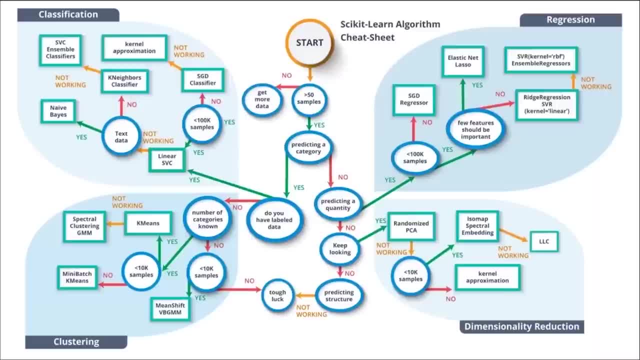 explains you which algorithm you should use and when. all it it's built in a decision tree format. Let's see how it is built. So, first condition: it will check whether you have 50 samples or not. If your samples are greater than 50, then it will move ahead. 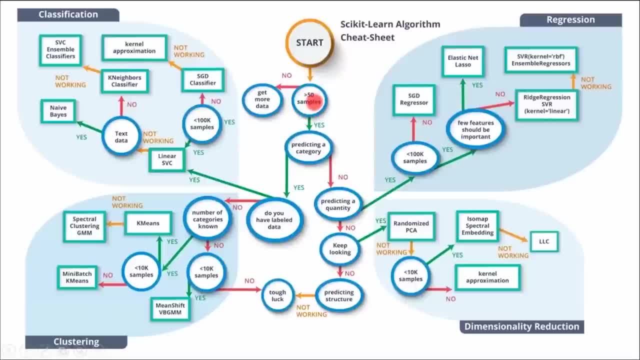 If it is less than 50, then you need to collect more data. If your sample is greater than 50. Then you have to decide whether you want to predict a category or not. If you want to predict a category, then further you will. 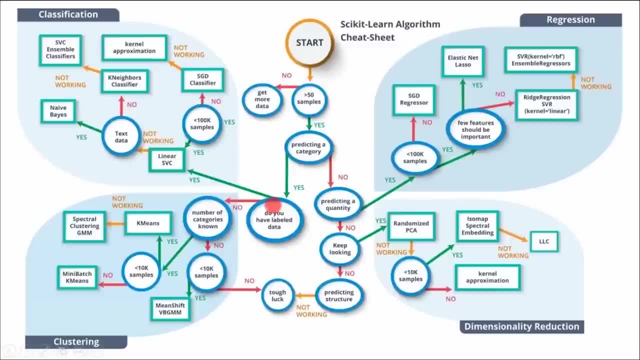 see that, whether you have label data or not, If you have label data, then that would be a classification algorithm problem. If you don't have the label data, then it would be a clustering problem. Now, if you don't want to predict a category, then what? 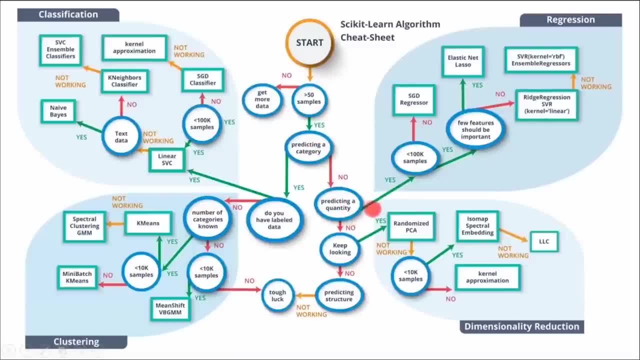 do you want to predict, predict a quantity? Well, if you want to predict a quantity, then in that case it would be a regression problem. If you don't want to predict a quantity and you want to keep looking further, than in that case you should go for. 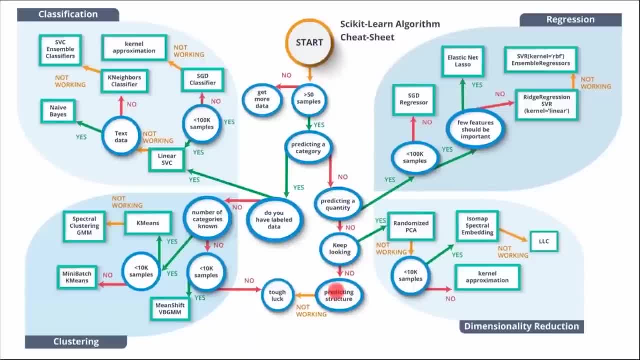 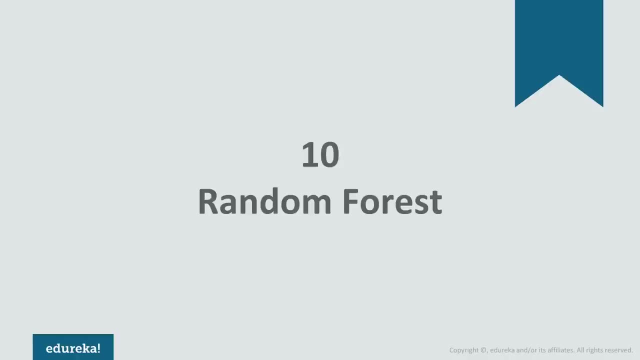 dimensionality reduction problems. and still, if you don't want to look and the predicting structure is not working, then you have tough luck for that. I hope this decision tree session clarifies all your doubt over decision tree algorithm. now we'll try to find out the answer to this particular question as to why we need. 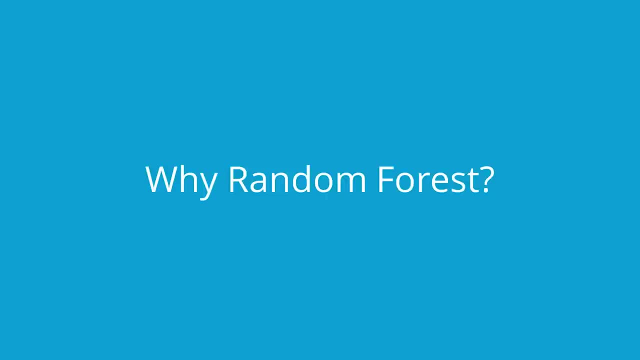 random forest, fine. so, like human beings, learn from the past experiences, so, unlike human beings, a computer does not have experiences. then how does machine takes decisions? where does it learn from? well, a computer system actually learns from the data, which represents some past experiences of an application domain. so 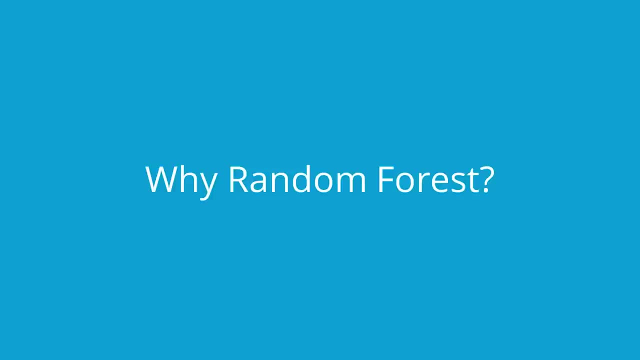 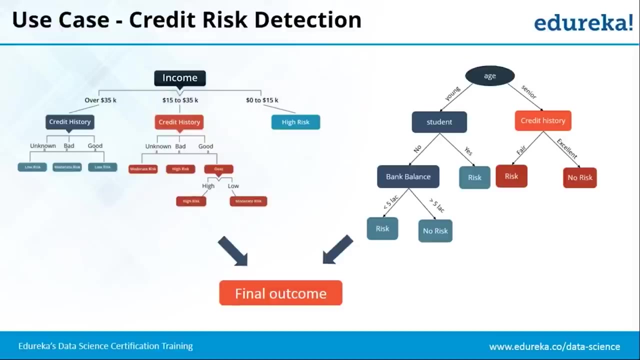 now let's see how random forest helps in building up the learning model with a very simple use case of credit risk detection. now, needless to say that credit card companies have a very nested interest in identifying financial transactions that are illegitimate and criminal in nature, and also- I would like to mention this point- 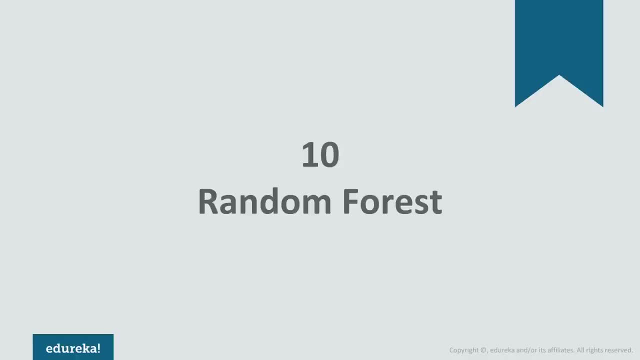 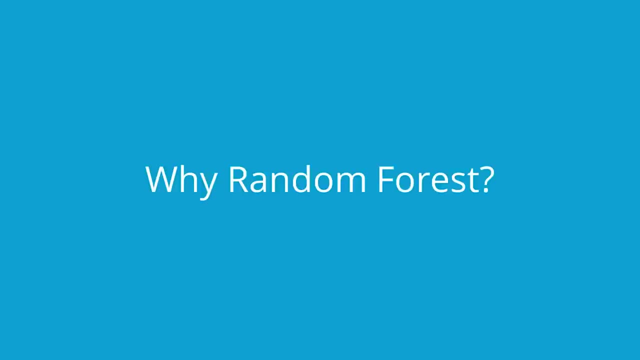 over decision tree algorithm. Now we'll try to find out the answer to this particular question as to why we need random forest. Fine, So, like human beings, learn from the past experiences. So, unlike human beings, a computer does not have experiences. 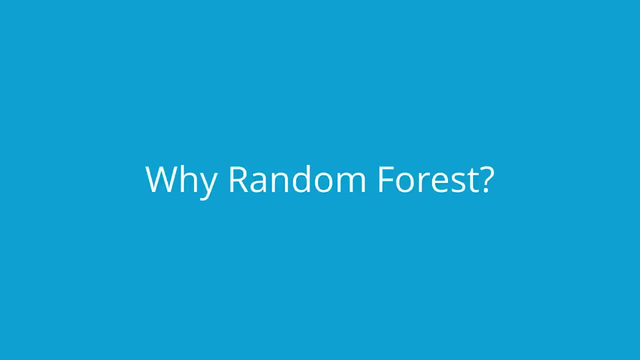 Then how does machine takes decisions? Where does it learn from? Well, a computer system actually learns from the data, which represents some past experiences of an application domain. So now let's see how random forest helps in building up the learning model with a very simple use case of credit risk detection. 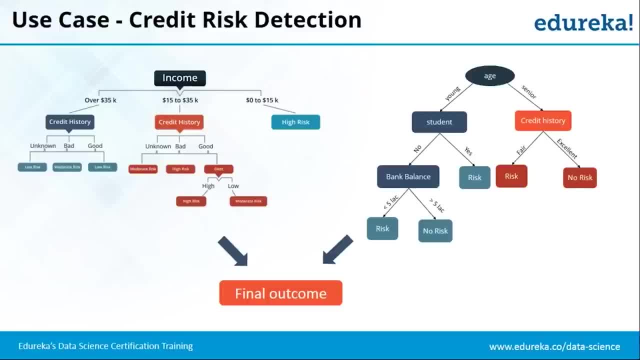 Now, needless to say, that credit card companies have a very nested interest in identifying financial transactions that are illegitimate and criminal in nature, And also, I would like to mention this point- that, according to the Federal Reserve payments study, Americans used credit cards to pay for 26.2 billion. 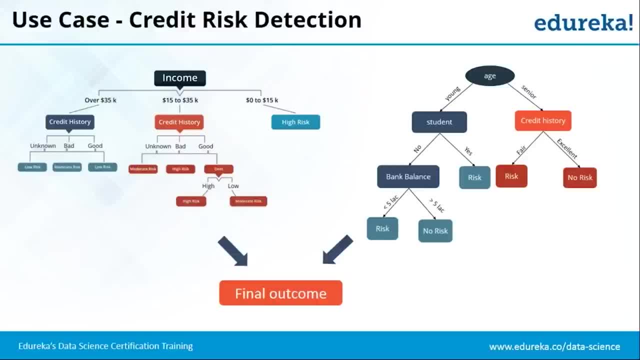 Purchases in 2012 and the estimated loss due to unauthorized transactions. that here was US 6.1 billion dollars. Now, in the banking industry, measuring risk is very critical because the stakes are too high, So the overall goal is actually to figure out who all can be. 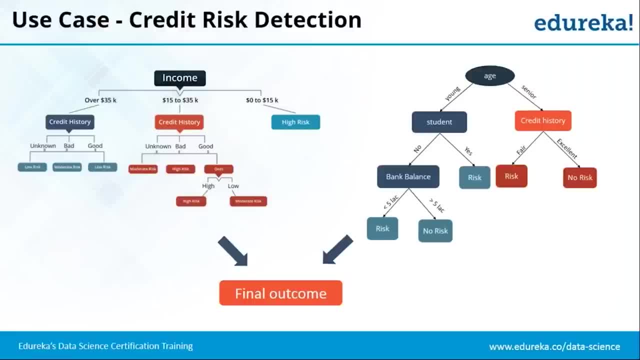 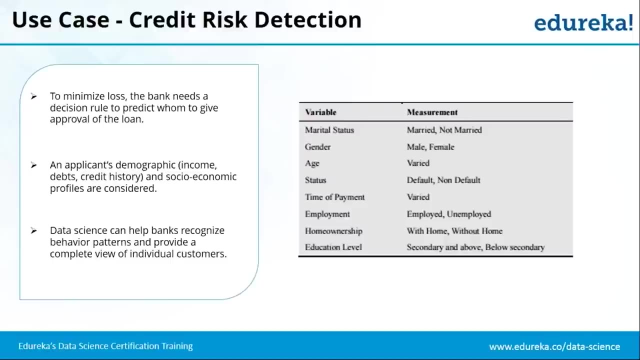 fraudulent before too much financial damage has been done. So for this, a credit card company receives thousands of applications for new cards, and each application contains information about an applicant right. So so here as you can see, that, from all those applications, what we can actually figure out is that predictor variables like what? 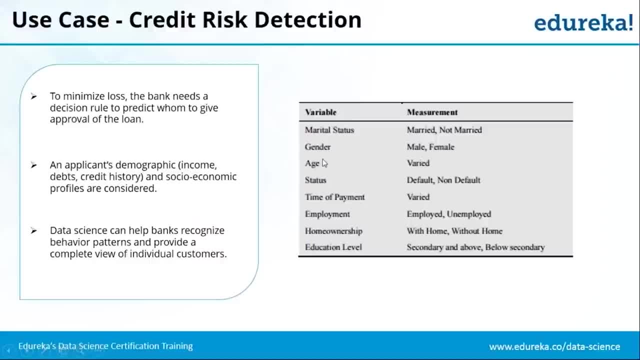 is the marital status of the person, What is the gender of the person, What is the age of the person and the status, which is actually whether it is a default pair or a non-default pair. so default payments Are basically when payments are not made in time and according. 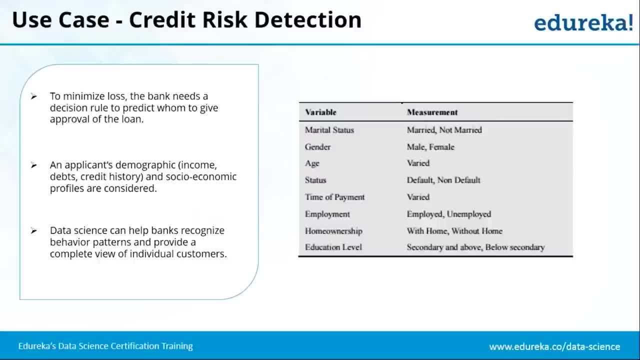 to the agreement signed by the cardholder. So now that account is actually set to be in the default. so you can easily figure out the history of the particular cardholder from this. then we can also look at the time of payment, whether he has been a regular pair or a non-regular one. 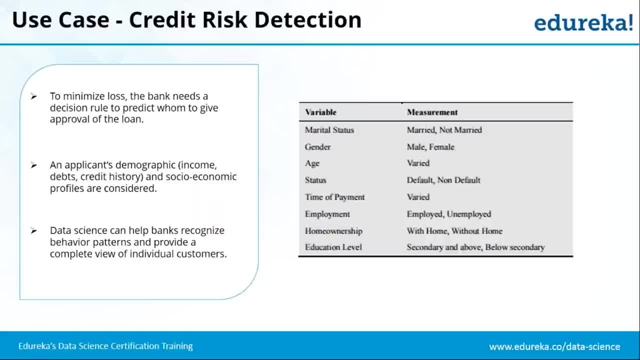 What is the source of income for that particular person, and so and so forth. So to minimize loss, the bank actually needs Certain decision rule to predict whether to approve a particular loan of that particular person or not. now here is where the random forest actually comes into the picture right now. 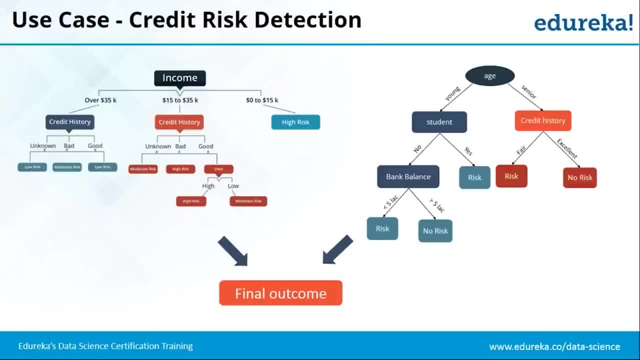 that, according to the Federal Reserve payments study, Americans used credit cards to pay for twenty six point two million purchases in 2012, and the estimated loss due to unauthorized transactions that year was us six point one billion dollars. now, in the banking industry, measuring risk is very critical, because the stakes are too high, so the overall goal is actually to 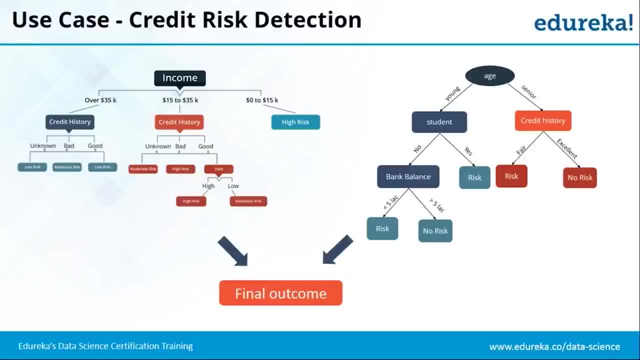 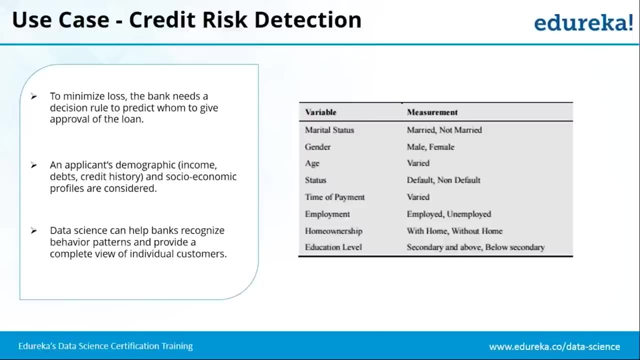 figure out who all can be fraudulent before too much financial damage has been done. so for this, a credit card company receives thousands of applications for new cards, and each application contains information about an applicant right. so so here as you can see that from all those applications, what we can actually figure out is our predictor variables. 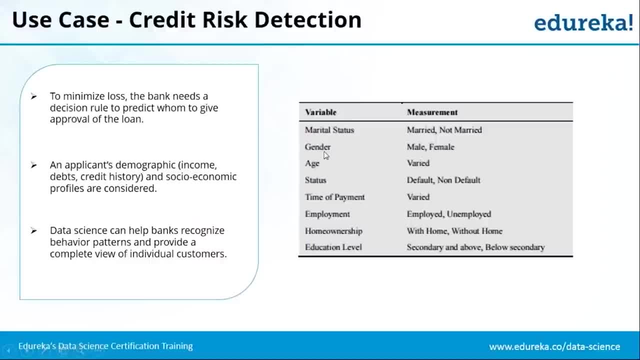 like: what is the marital status of the person, what is the gender of the person, what is the age of the person and the status, which is actually whether it is a default pair or a non default pair. so default payments are basically when payments are not made in time and according to the agreement signed by the 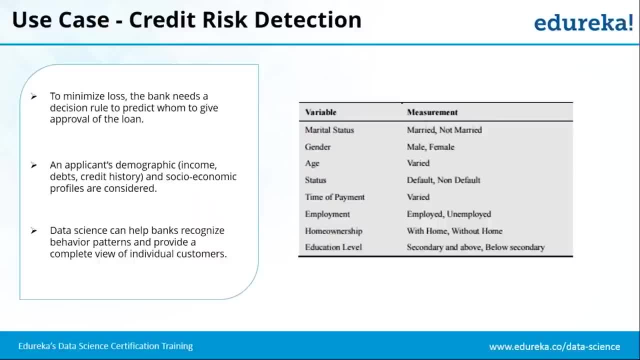 cardholder. so now that account is actually set to be in the default. so you can see that the default account is actually set to be in the default. so you can easily figure out the history of the particular cardholder from this. then we can also look at the time of payment, whether he has been a regular. 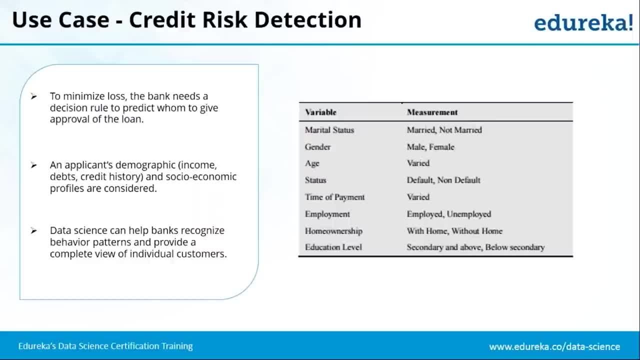 pair or a non regular one, what is the source of income for that particular person, and so and so forth. so to minimize loss, the bank actually needs certain decision rule to predict whether to approve a particular loan of that particular person or not. now here is where the random forest actually comes. 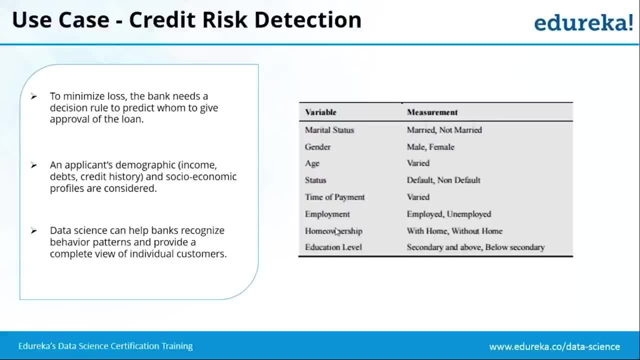 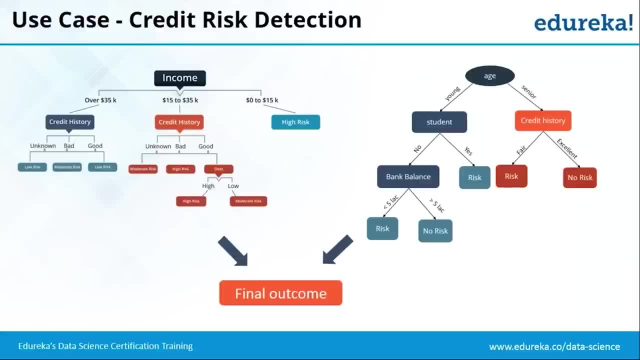 into the picture right now. let's see how random forest can actually help us in this particular scenario. now we have taken randomly two parameters out of all the predictive variables that we saw previously. now we have taken two predictor variables here. the first one is the income and the second one is the age right and similarly. 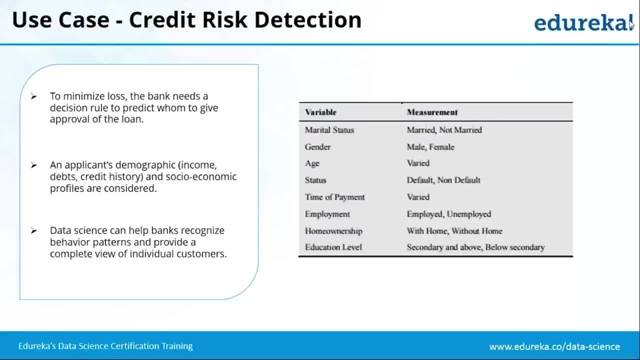 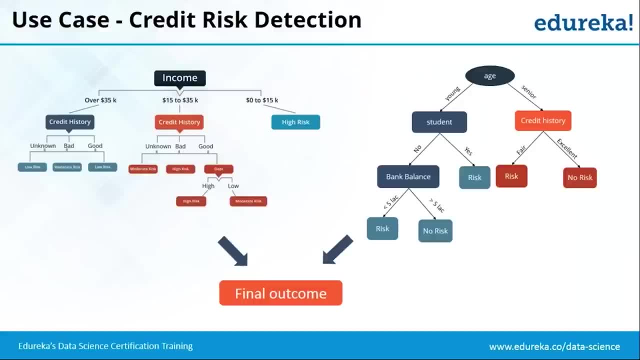 Let's see how random Forest can actually help us in this particular scenario. Now we have taken randomly two parameters out of all the predictive variables that we saw previously. Now we have taken two predictor variables here. The first one is the Income and the second one is the age right and similarly. 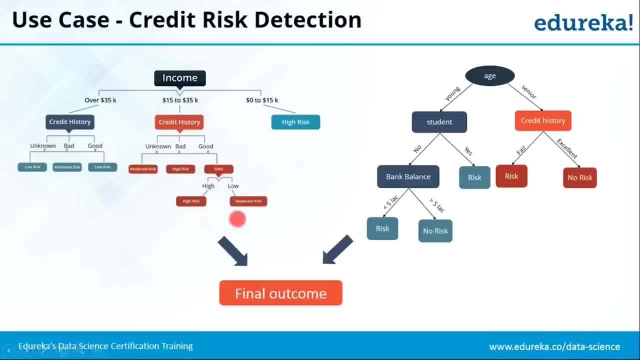 parallely to decision trees have been implemented upon those predicted variables, And let's first assume the case of the income variable, right. So here we have divided our income into three categories, The first one being the person earning over $35,000. second from: 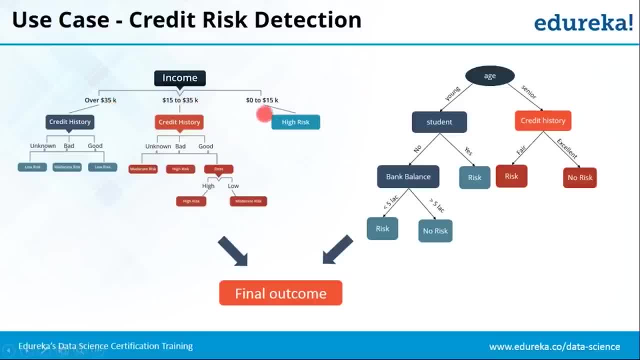 15 to $35,000, the third one earning in the range of zero to $15,000.. Now, if a person is Earning over $35,000, which is a pretty good income, pretty decent. So now we'll check out for the credit history and here the probability. 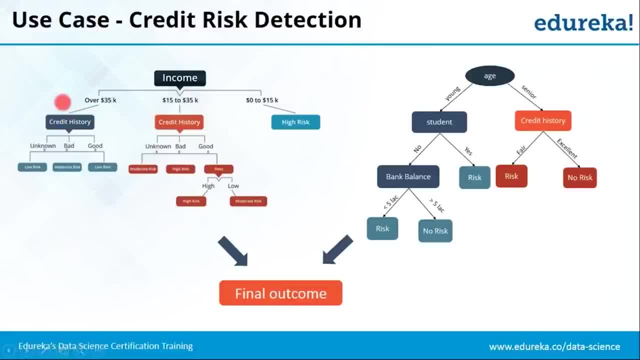 is that if a person is earning a good amount, then there is very low risk that he won't be able to pay back already earning goods. So the probability is that his application of loan will get approved right. So there is actually low risk or moderate risk. 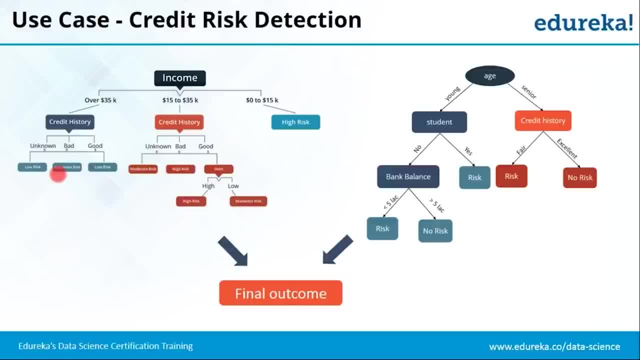 There's no real issue of higher risk. as such, We can approve the applicants request here. Let's move on and watch out for the second category, where the person is actually earning from 15 to $35,000 right now. here the person may or may not pay back. 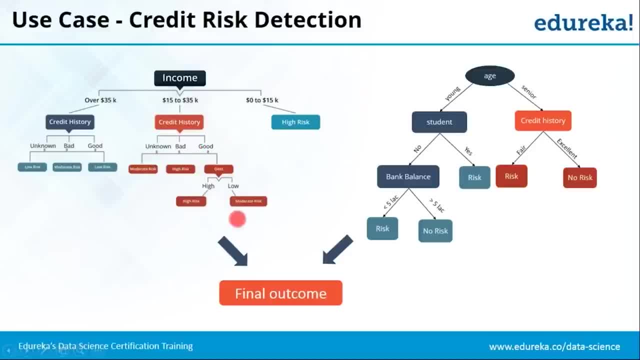 parallelly, two decision trees have been implemented upon those predicted variables. let's first assume the case of the income variable, right? so here we have divided our income into three categories, the first one being the person earning over $35,000. second, from 15 to $35,000. the third one, earning in the range of 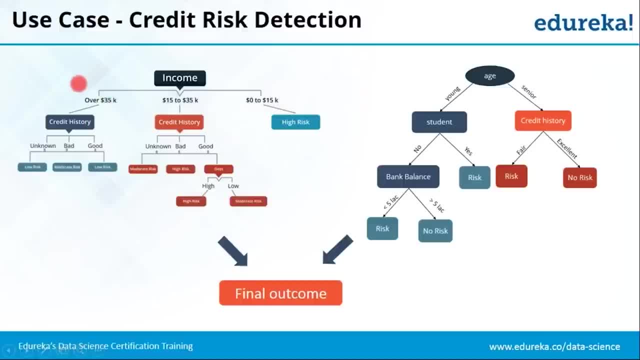 zero to $15,000. now if a person is earning over $35,000, which is a pretty good income, pretty decent. so now we'll check out for the credit history. now the here the probability is that if a person is earning a good amount, then there is 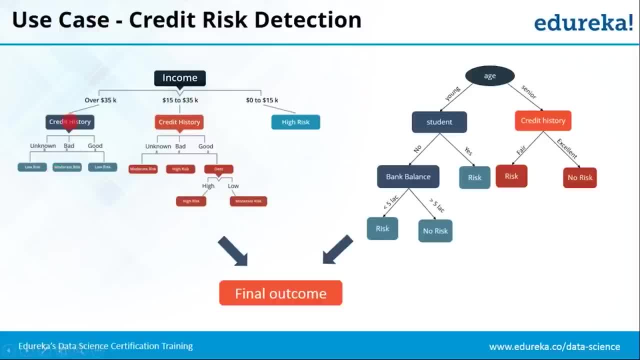 very low risk that he won't be able to pay back already earning goods, so the probability is that his application of loan will get approved right. so there is actually low risk or moderate risk, but there's no real issue of higher risk. as such, we can approve the applicants request here. now let's move on and watch. 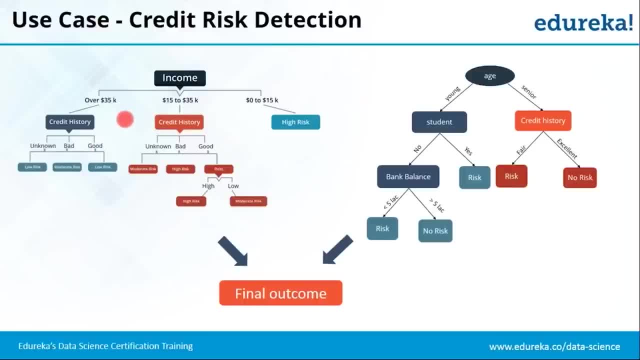 out for the second category, where the person is actually earning from fifteen to thirty five thousand dollars right now. here the person may or may not pay back. so in such scenarios will look for the credit history as to what has been his previous history. now, if his previous history has been bad, like he has been a 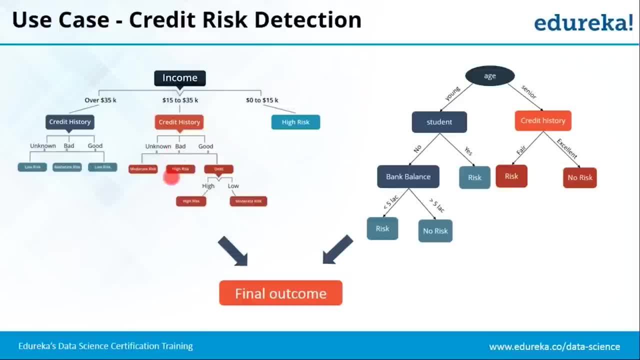 defaulter in the previous transactions will definitely not consider approving his request and he'll be at the high risk end, which is not good for the bank. if the previous history of that particular applicant is really good, then we will- just to clarify a doubt- will consider. 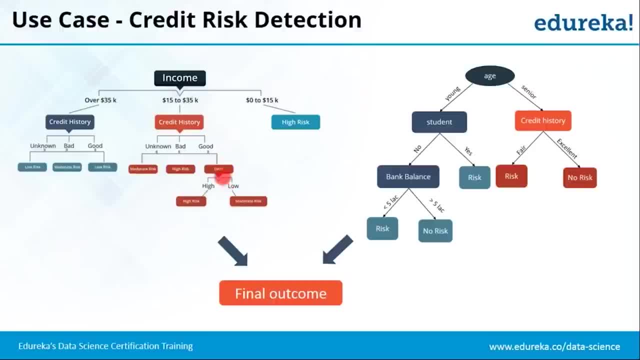 another parameter as well that will be a debt. if he's already in really high debt then the risks again increases and there are chances that he might not pay repay in the future. so here will not accept the request of the person having high debt. if the person is in the low debt and he has been a good pair in his past history. 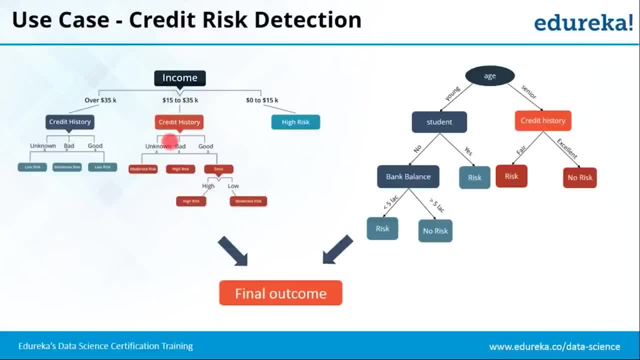 So in such scenarios will look for the credit history as to what has been his previous history of. if his previous history has been bad, like he has been a defaulter In the previous transactions, will definitely not consider approving his request and he'll be at the high risk end, which is not good for. 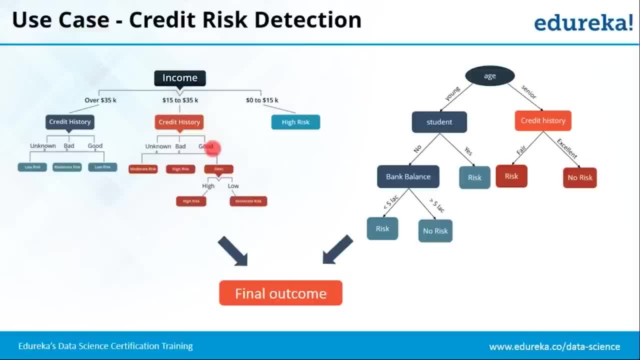 the bank. If the previous history of that particular applicant is really good, then we will- just to clarify a doubt- will consider another parameter as well. that will be adept if he's already in really high depth and the risks again increases and there are chances that he might. 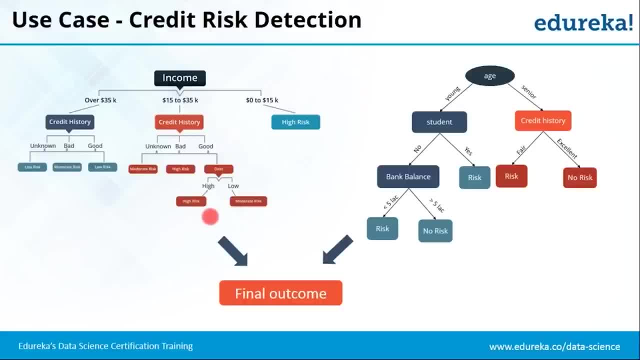 Not pay repay in the future. So here will not accept the request of the person having high depth. If the person is in the low depth and he has been a good pair in his past history, then there are chances that he might pay back and we can. 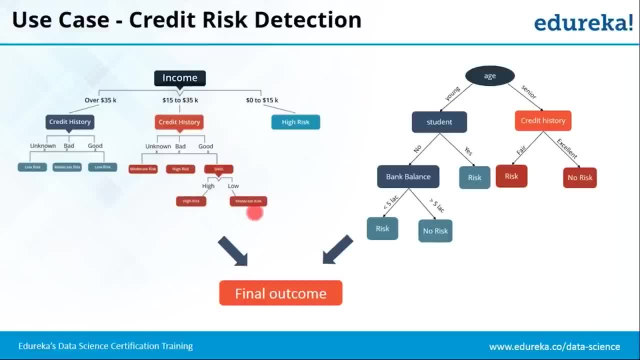 consider approving the request of this particular applicant. And let's look at the third category, which is a person earning from zero to $15,000.. Now, this is something which actually raises I pro, and this person will actually lie in the category of high risk. 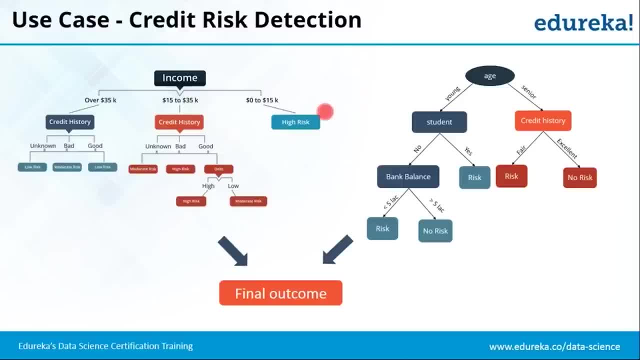 All right. so the probability is that his application of loan will probably get rejected. Now we'll get one final outcome from this income parameter. right Now let us look at our second variable, that is, age, which will lead into the second decision tree. 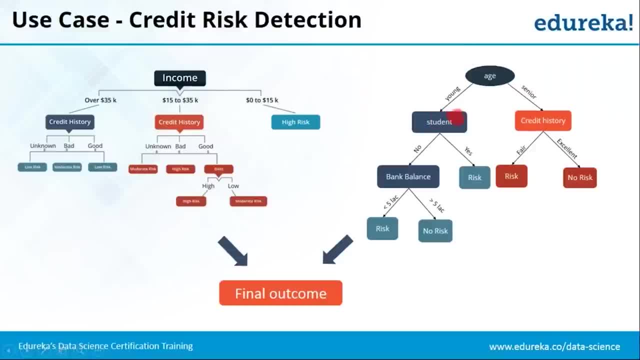 Now let us say: if the person is young, right, So now we look forward To if it is a student. now, if it is a student, then the chances are high that he won't be able to repay back because he has no earning. 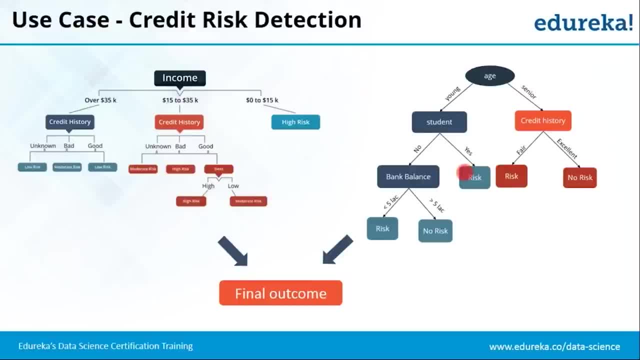 source right. So here the risks are too high and probability is that his application of loan will get rejected. fine, Now if the person is young and he's not a student, then we'll probably go on and look for another variable, that is, bank balance. 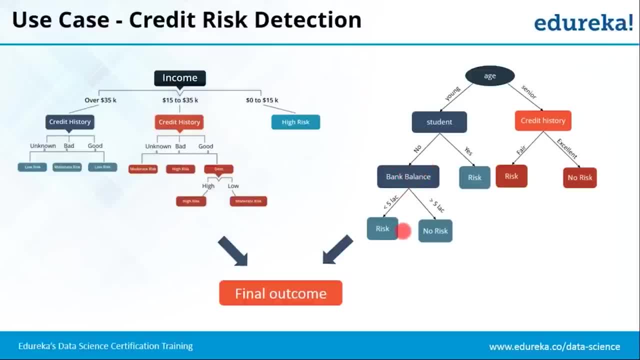 Now let's look if the bank balance is less than five lakhs. So again, the risk arises and the Probability is that his application of loan will get rejected. Now, if the person is young, is not a student and his bank balance of 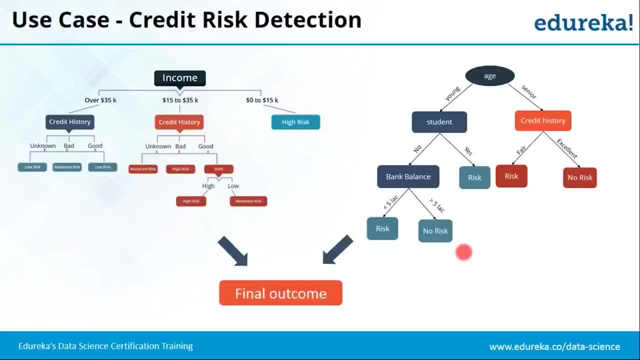 greater than five lakhs, is got a pretty good and stable bank balance, Then the probability is that his loan of application will get approved off. Now let us take another scenario. if he's a senior, right? So if he's a senior will probably go and check out for his credit. 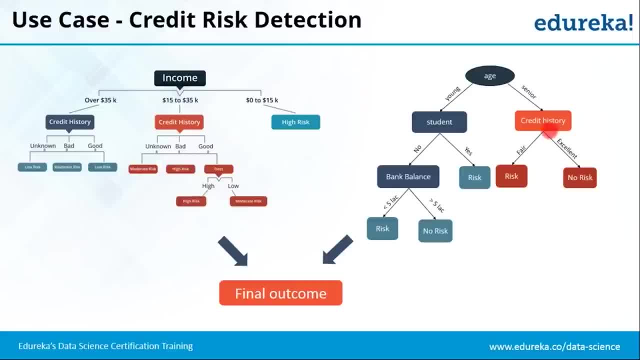 history, How well has he been in his previous transactions, What kind of a person he's like, whether he's a defaulter or he's a non-default, or now, if he's a very fair kind of person in his previous transactions, then again the risk arises and the probability of his 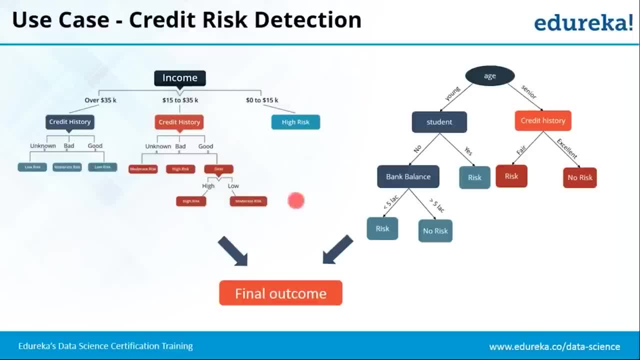 then there are chances that he might pay back and we can consider approving the request of this particular applicant. now let's look at the third category, which is a person earning from zero to fifteen thousand dollars. now, this is something which actually raises eyebrow, and this person will actually lie in the category. 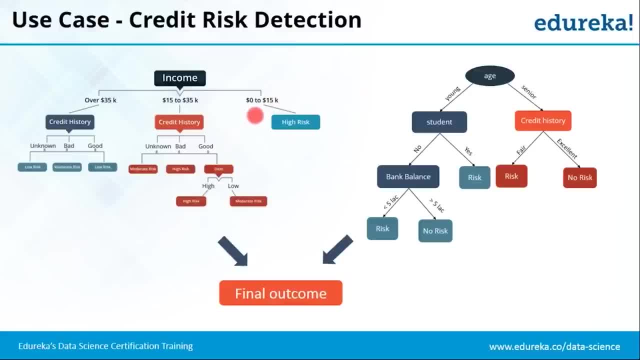 of high risk, all right. so the probability is that his application of loan will probably get rejected. now we'll get one final outcome from this income parameter. right now let us look at our second variable, that is, age, which will lead into the second decision tree. now let us say: if the person is young, right. so now we'll look forward to if it. 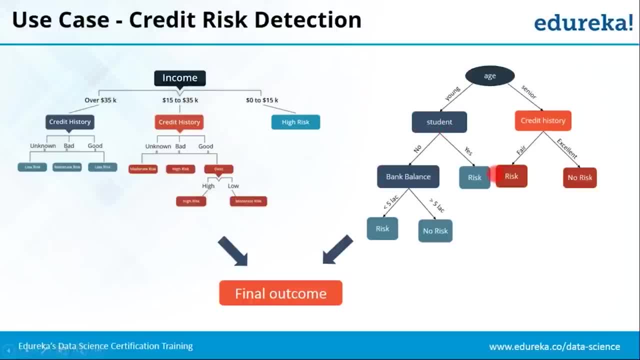 is a student now? if it is a student, then the chances are high that he won't be able to repay back because he has no earning source right. so here the risks are too high and the probability is that his application of loan will get rejected. fine now if the person is young and he's not a student. 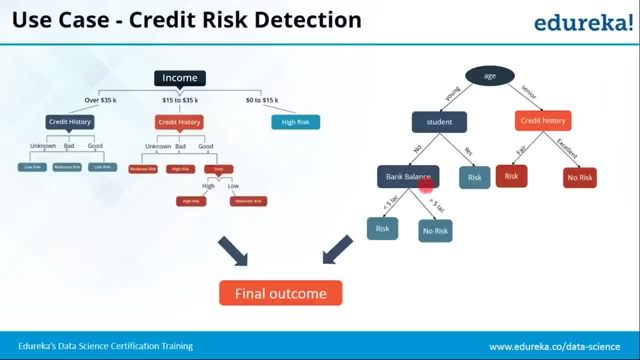 then we'll probably go on and look for another variable, that is, bank balance. now let's look if the bank balance is less than five lakhs. so again, the risk arises and the probability is that his application of loan will get rejected. now, if the person is young, he is not a student. 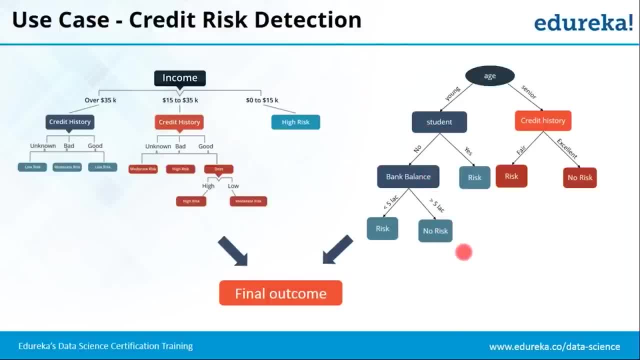 and he has a bank balance of greater than five lakhs, he's got a pretty good and stable bank balance. then the probability is that his own of applications will get approved off. now let us take another scenario. if he is a senior, right. so if he is a senior, we'll. 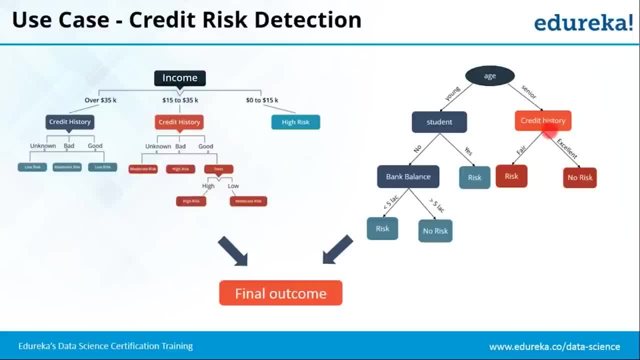 probably go and check out for credit history. how well has he been in his previous transactions, what kind of a person he is like, whether he is a defaulter or he is a non-defaulter. now, if he is a very fair kind of person, he will be able to get approved for any of his previous. 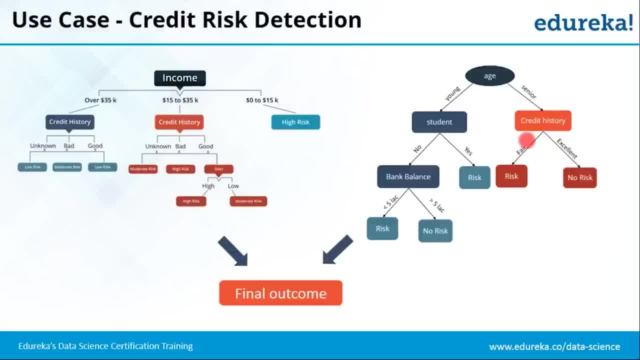 transactions, whether he is a default or he is a non-defaulter. now, if he is a very fair of person in his previous transactions, then again the risk arises and the probability of his application getting rejected actually increases right now. if he has been an excellent person as per his transactions in the previous history, 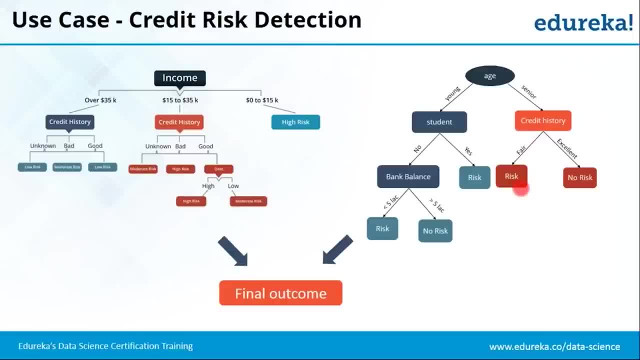 application getting rejected actually increases right now if he has been an excellent person as per his transactions in the previous history. So now again here there is least risk and the probabilities that his application of loan will get approved. So now here. these two variables, income and age, have led to two different. 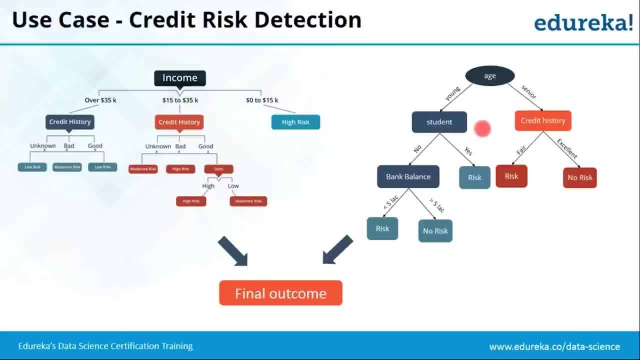 decision trees right, and these two different decision trees actually led to two different results. Now, what random forest does is it will actually compile these two different results from these two different decision trees and then, finally, it will lead to a final outcome. That is how random forest actually works, right? 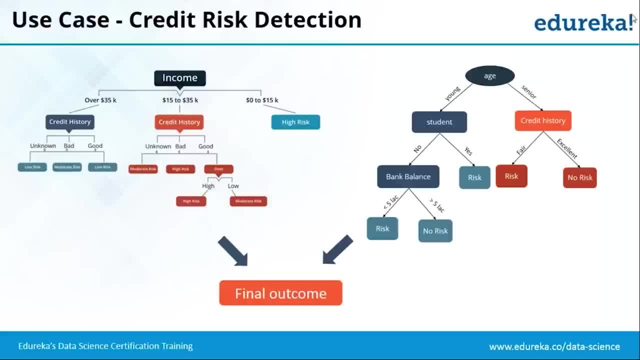 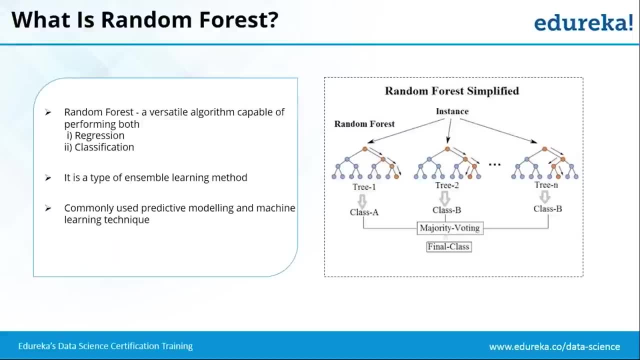 So that is actually the motive of the random forest. Now Let us move forward and see what is random forest. right, You can get an idea of the mechanism from the name itself: random forest. So a collection of trees is a forest. That's why called forest, probably, and here also the trees are actually. 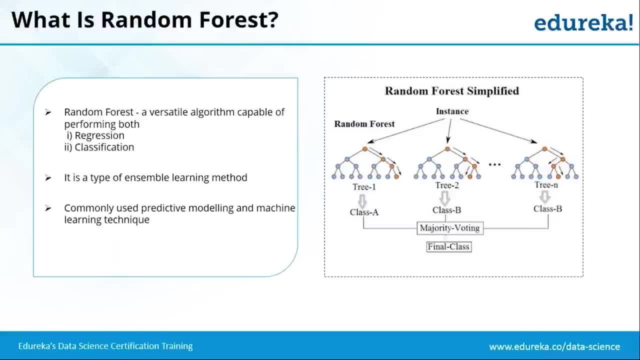 because being trained on subsets which are being selected at random and therefore they are called random forests. So a random forest is a collection or an ensemble of decision trees. Right Here a decision tree is actually built using the whole data set, considering all features, but actually in random forest, only a fraction of the number of 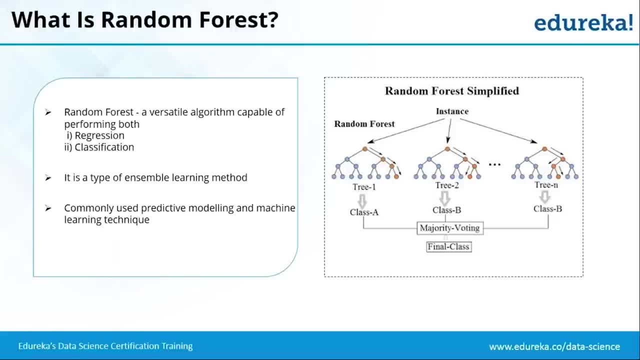 rows is selected, and that, too, at random, and a particular number of features, which are actually selected at random, are trained upon, and that is how the decision trees are built upon, right? So, similarly, number of decision trees will be grown and each decision tree will result. 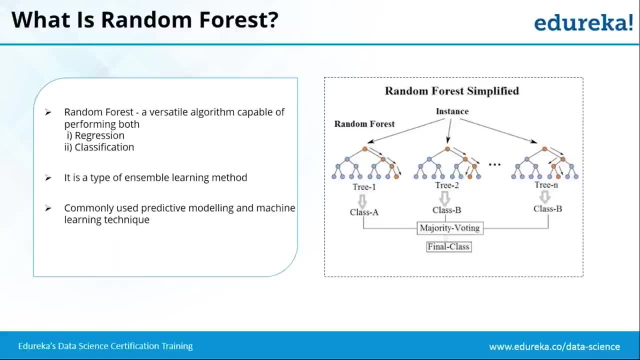 into a certain final outcome and random forest will do nothing but actually just compile the results of all those decision trees to bring out the final result. As you can see in this particular figure that a particular instance actually has resulted into three different decision trees, right. 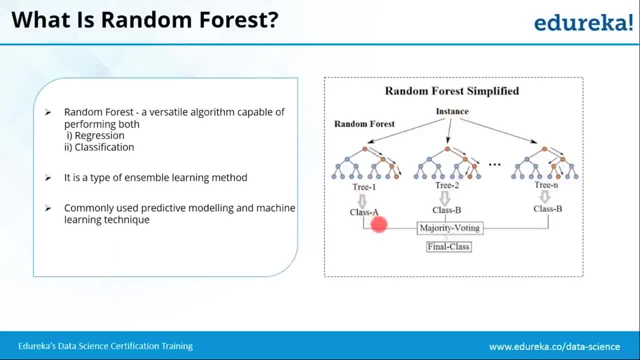 So now tree one results into a final outcome called class A, and tree two results into class B. Similarly, tree three results into class B. So random forest will compile the results of all these decision trees And it will go by the call of the majority voting. 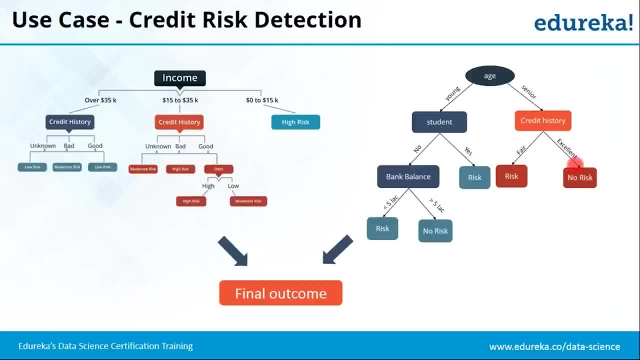 so now again, here there is least risk and the probabilities that his application of loan will get approved. so now here, these two variables, income and age, have led to two different decision trees. right, and these two different decision trees actually lead to two different results. now, what random forest. 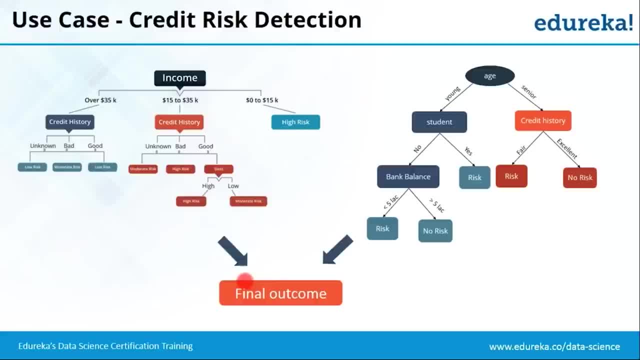 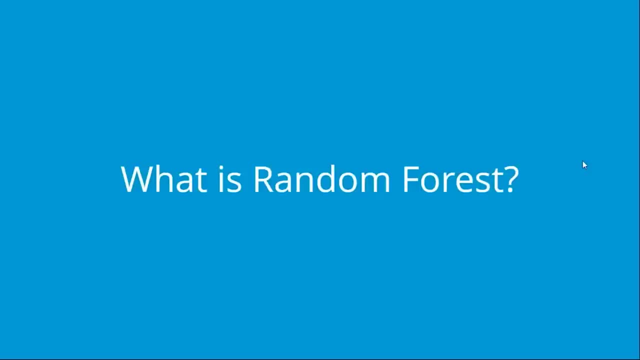 does is it will actually compile these two different results from these two different decision trees and then, finally, it will lead to a final outcome. that is how random forest actually works, right? so that is actually the motive of the random forest. now let us move forward and see what is. 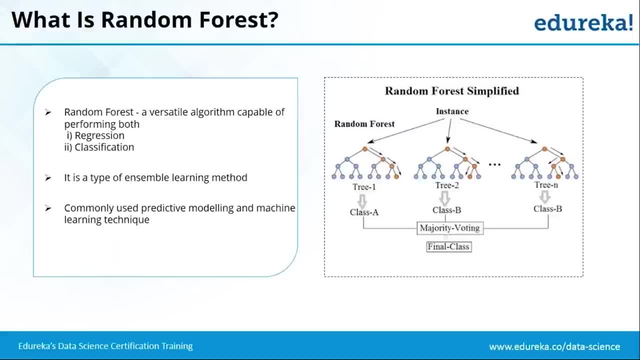 random forest. you right, you can get an idea of the mechanism from the name itself: random forests. so a collection of trees is a forest. that's why called forest, probably, and here also the trees are actually because being trained on subsets which are being selected at random, and therefore they are called random forests. 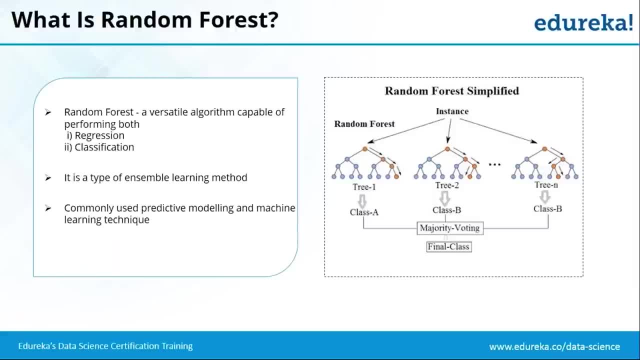 so a random forests is a collection or an ensemble of decision trees. right here, a decision tree is actually built using the whole data set, considering all features, but actually in random forest, only a fraction of the number of rows is selected, and that too, at random and a particular number of features which are 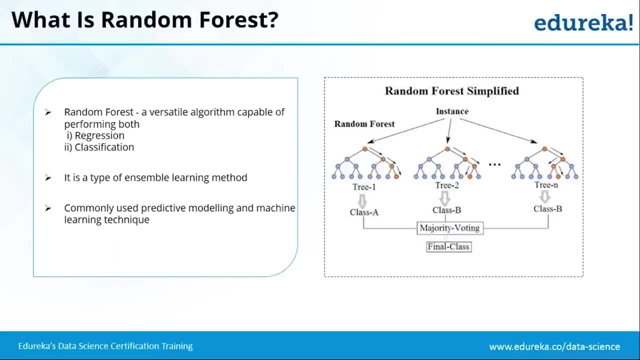 actually selected at random, are trained upon, and that is how the decision trees are built upon, right? so, similarly, number of decision trees will be grown and each decision tree will result into a certain final outcome, and random forests will do nothing but actually just compile the results of all. 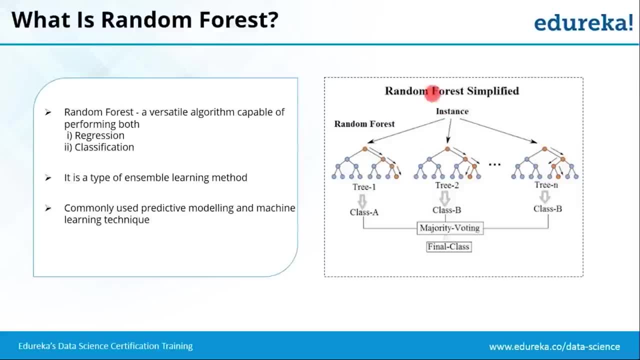 those decision trees to bring out the final result. as you can see in this particular figure that a particular instance actually has resulted into three different decision trees. right, so now? tree one results into a final outcome called class A, and tree two results into class B. similarly, tree three. 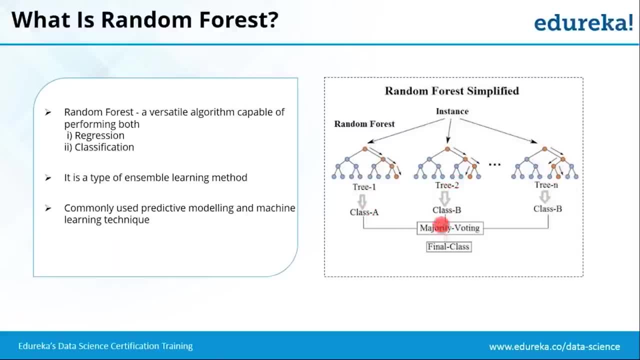 results into class B. so random forest will compile the results of all these decision trees and it will go by the call of the majority voting now, since here two decision trees have actually voted into the favor of the class B, that is, decision tree two and three, therefore the 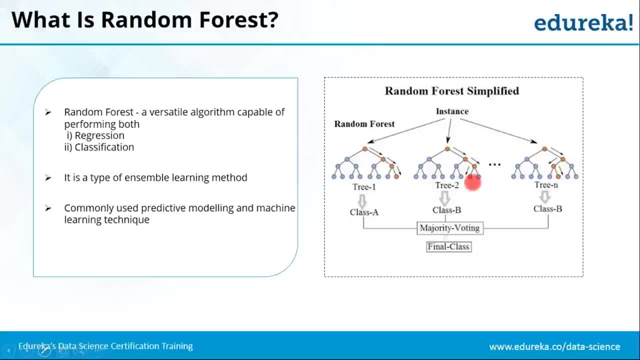 Now, since here, two decision trees have actually voted into the favor of the class B, that is, decision tree two and three. Therefore, the final outcome will be in the favor of the class B, and that is how random forest actually works upon. Now, one really beautiful thing about this particular algorithm is that it is one of the versatile 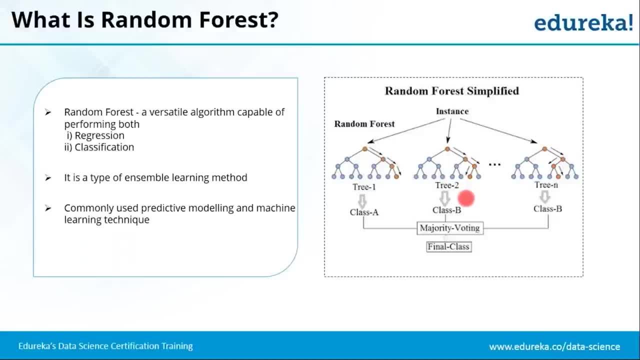 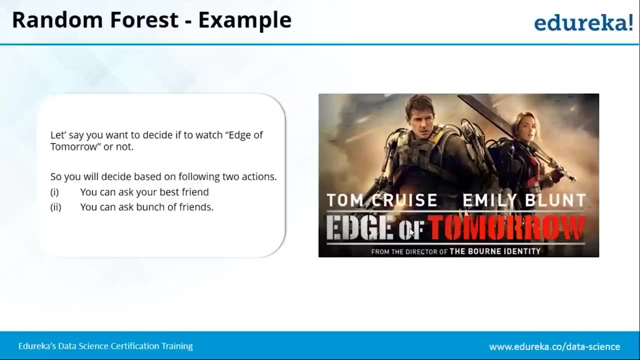 algorithms which is capable of performing both regression as well as classification. Now let's try to understand random forest further with a very beautiful example. All right, This is my favorite one. So let's say, you want to decide if you want to watch Edge of Tomorrow or not. right? 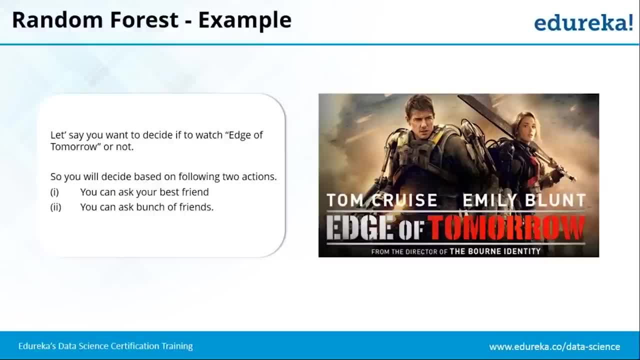 So in this particular scenario, you will have two different actions to work upon. Either you can just straight away go to your best friend, ask him about, all right, whether should I go for Edge of Tomorrow or not. Will I like it, Like this movie? or you can ask a bunch of friends and take their opinion consideration. 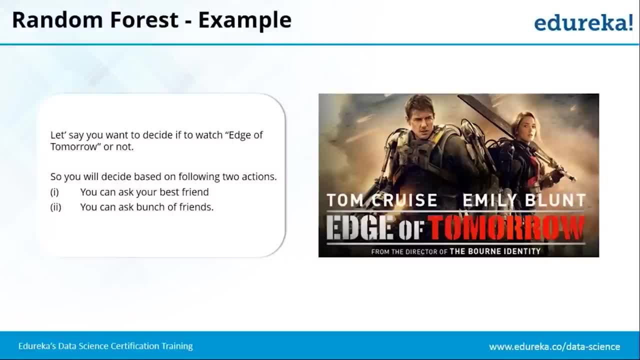 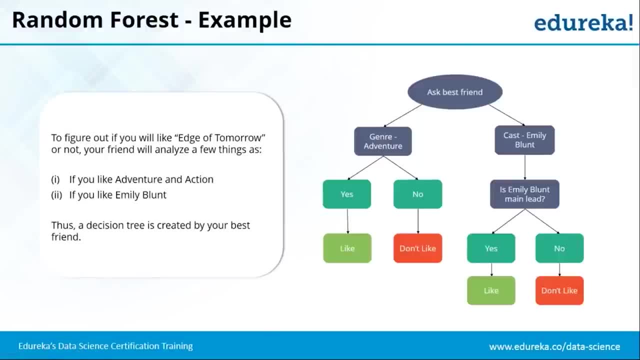 and then, based on the final result, you can go out and watch Edge of Tomorrow, right? So now let's just take the first scenario, So, where you go to your best friend, ask about whether you should go out to watch Edge of Tomorrow or not. 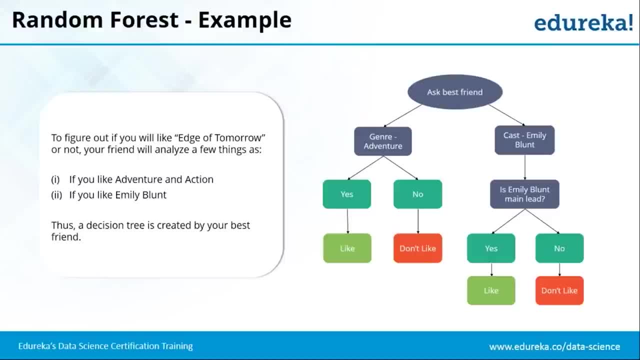 So your friend will probably ask you a certain questions, like the first one being here Jonah. So let's say your friend asks you if you really like the adventurous kind of movies or not. So you say, yes, definitely I would love to watch Adventure kind of movie. 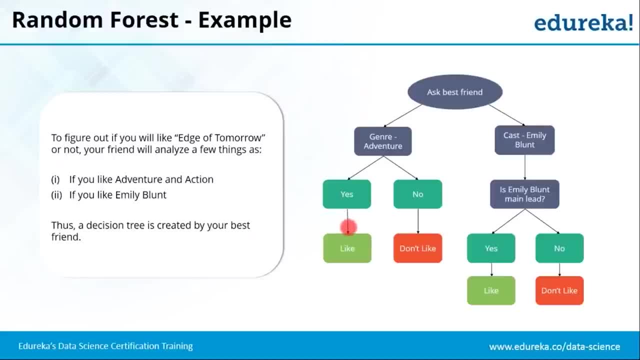 So the probabilities that you will like Edge of Tomorrow as well, since Edge of Tomorrow is also a movie of Adventure and sci-fi, kind of Jonah right. So let's say you do not like the Adventure Jonah movie, So then again the probability reduces that you might really not like Edge of Tomorrow. 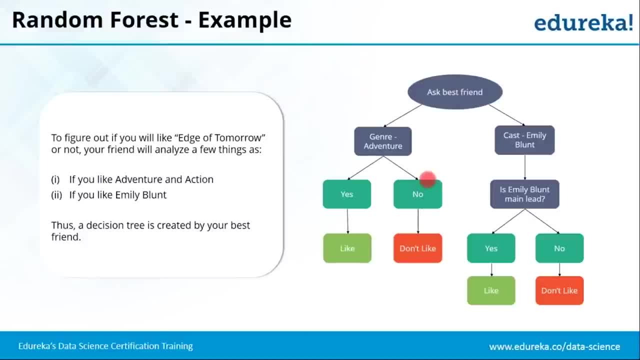 right, So from here you can come to a certain conclusion. right, Let's say, your best friend puts you into another situation where he'll ask you: or do you like Emily Blunt? and you say definitely, I like Emily Blunt. and then he puts another question. 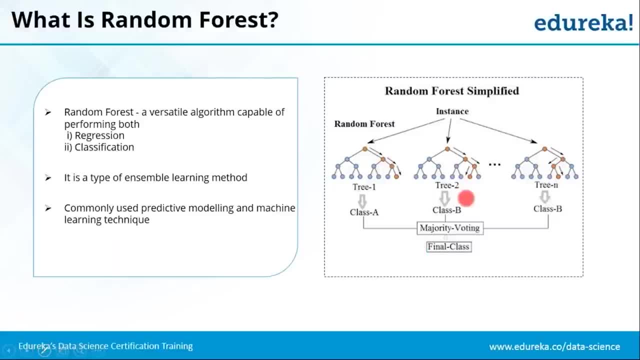 final outcome will be in the favor of the class B, and that is how random forests actually works upon. now, one really beautiful thing about this particular algorithm is that it is one of the versatile algorithms which is capable of performing both regression as well as classification. now let's try. 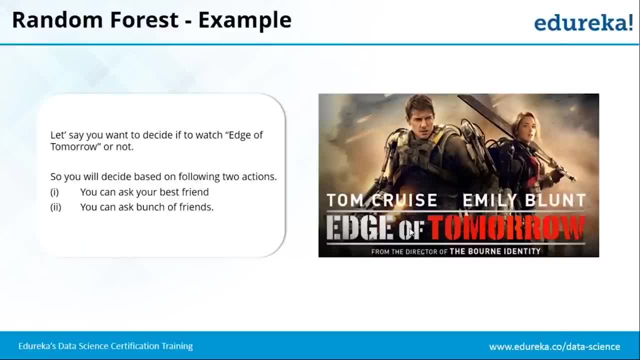 to understand random forests further with a very beautiful example. all right, this is my favorite one. so let's say you want to decide if you want to watch edge of tomorrow or not, right? so in this particular scenario, you will have two different actions to work upon. either you can just straight away go to your 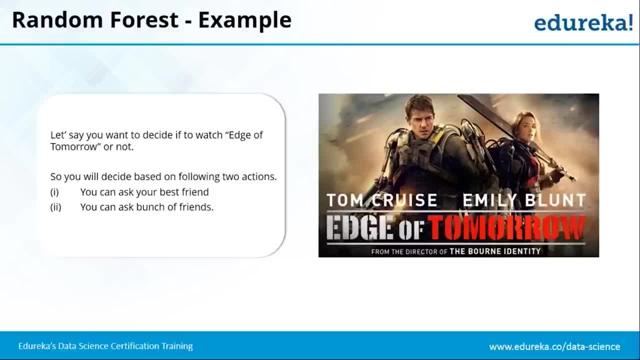 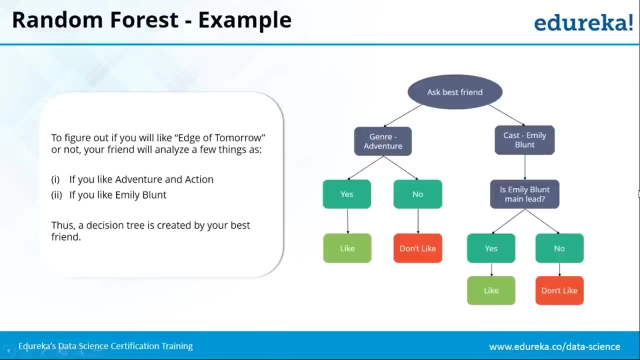 best friend, ask him about, all right, whether should I go for edge of tomorrow or not. will I like this movie? or you can ask a bunch of friends and take their opinion consideration and then, based on the final result, you can go out and watch edge of tomorrow, right? so now let's just take the first scenario. 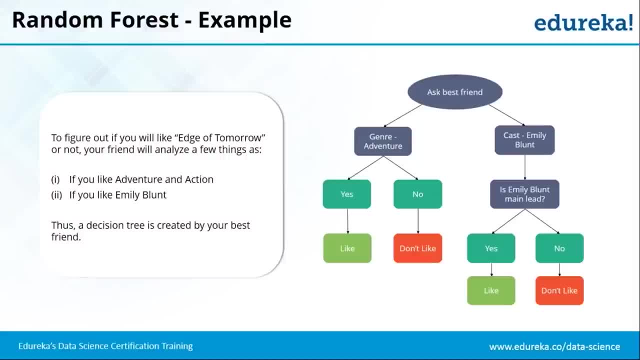 so where you go to your best friend, ask about whether you should go out to watch edge of tomorrow or not. so your friend will probably ask you certain questions, like the first one being here Jonah. so so let's say your friend asks you if you really like. 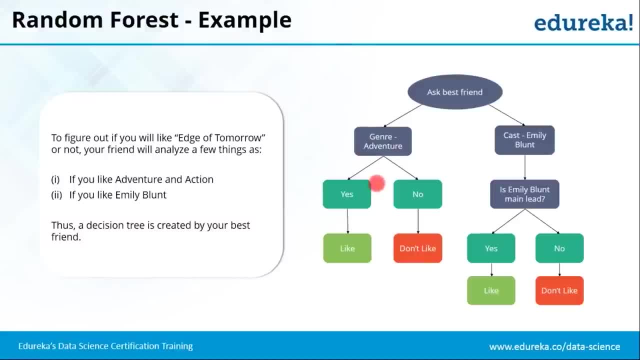 the adventurous kind of movies or not. so you say yes, definitely I would love to watch adventure kind of movie. so the probability is that you will like edge of tomorrow as well, since edge of tomorrow is also a movie of adventure and sci-fi kind of genre. right? so let's say you do not like the adventure genre. 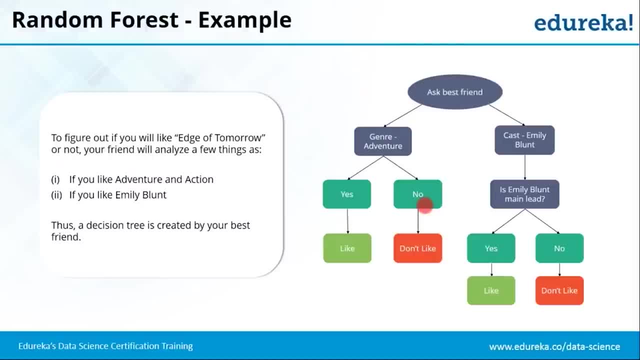 movie. so then again, the probability reduces that you might really not like edge of tomorrow. right, so from here you can come to a certain conclusion that the best friend likes this movie. and if you say, yes, you like this movie at the end of the cast, that is the best friend. I think there will not be any funny. 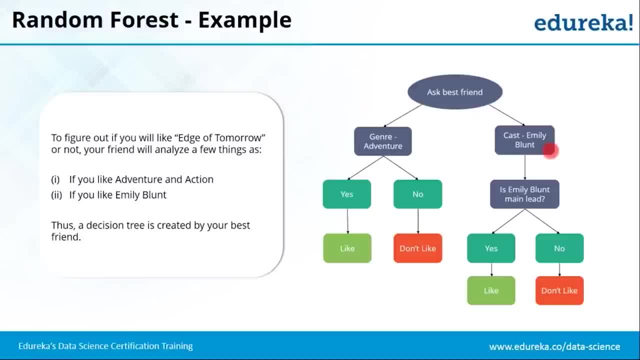 consequences. right, let's say, your best friend puts you into another situation where he'll ask you: all right, do you like Emily Blunt? and you say definitely, I like Emily Blunt. and then he puts another question to you: do you like Emily Blunt to be in the main lead? and you say yes and again. 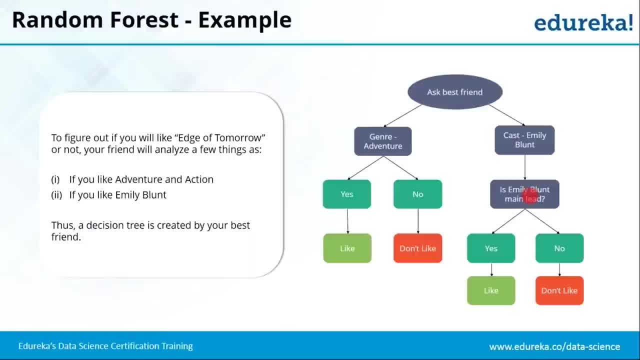 to you: Do you like Emily Blunt to be in the main lead? and you say yes, and again the probability arises that you will definitely like Edge of Tomorrow as well, because Edge of Tomorrow's has the Emily Blunt in the main lead cast. so and if you say, oh, I do not like Emily Blunt, then 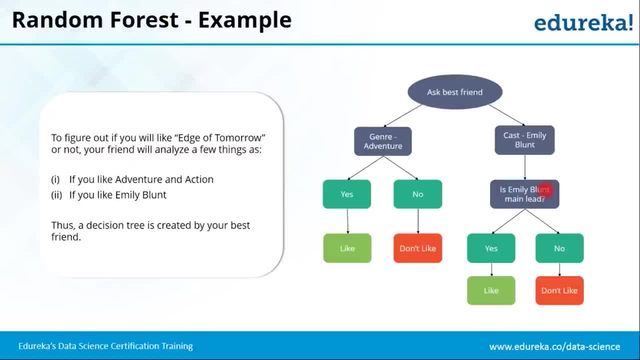 again, the probability reduces that you would like Edge of Tomorrow too, right? So this is one way where you have one decision tree and your final outcome. your final decision will be based on your one decision tree, or you can say: your final outcome will be based 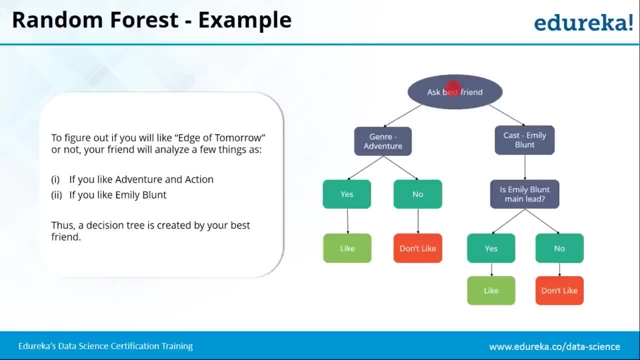 on just one friend Now, definitely, you're not really convinced. You want to consider the options of your other friends also so that you can make very precise and crisp decision. right, You go out and you approach some other bunch of friends of yours. 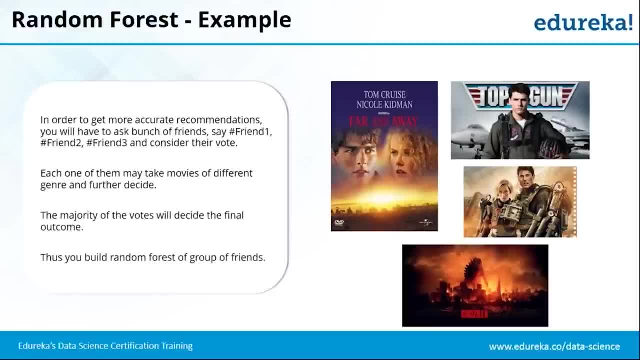 So now, let's say you go to three of your friends and you ask them the same question: whether I would like to watch Edge of Tomorrow or not. So you go to an approach, three of your friends, friend one, friend two and friend three. now you will consider each of theirs vote and then you will. 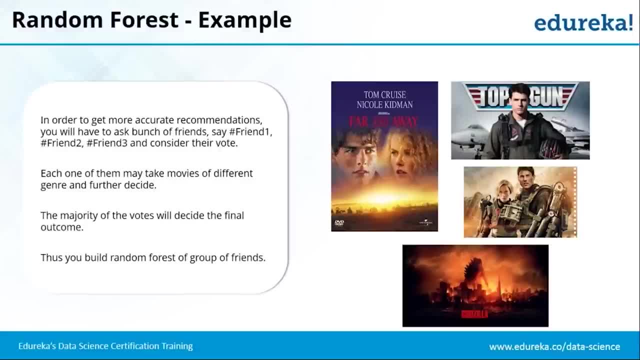 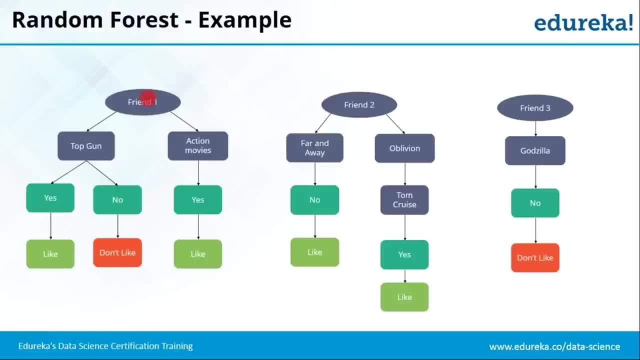 Your decision now will be dependent on the compiled results of all of your three friends right Now here. let's say you go to your first friend and you ask him whether you would like to watch Edge of Tomorrow or not, and your first friend puts you to one question. 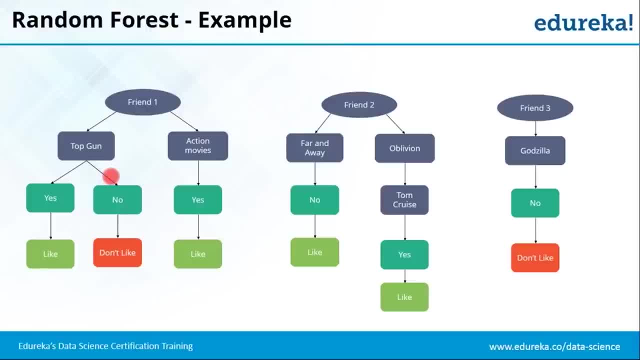 Did you like Top Gun? and you say, yes, definitely, I did like the movie Top Gun and the probabilities that you would like Edge of Tomorrow as well, because Top Gun is actually a military action drama, Which also Tom Cruise. So now again, the probability rises that, yes, you will like Edge of Tomorrow as well. 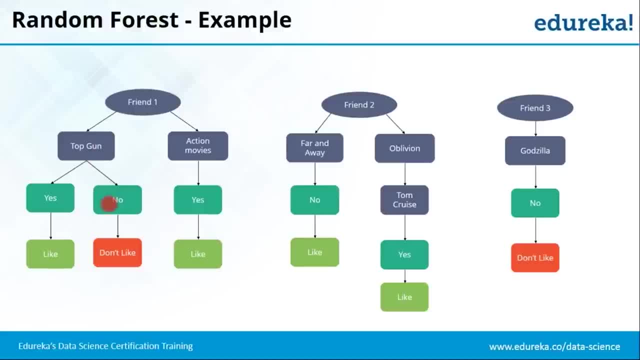 And if you say no, I didn't like Top Gun, then again, the chances are that you wouldn't like Edge of Tomorrow, right? Then another question that he puts you across is that: do you really like to watch action movies? and you say, yes, I would love to watch them. 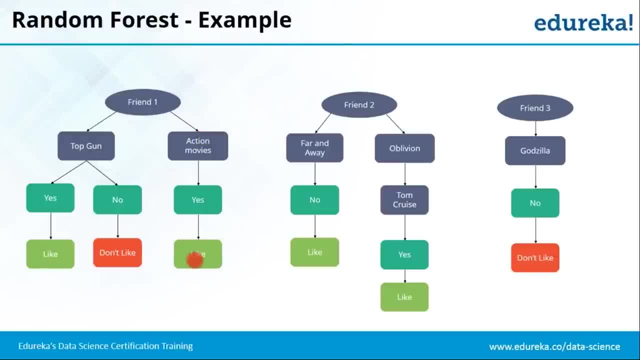 Then again, the chances are that you would like to watch Edge of Tomorrow. So from your friend one, you can come to one conclusion, I hear, since The ratio of liking the movie to don't like is actually two is to one. So the final result is actually: you would like Edge of Tomorrow. 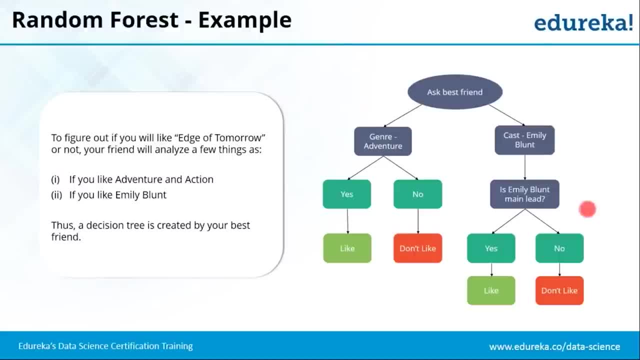 the probability arises that you will definitely like edge of tomorrow as well. if you say, oh, I do not like Emily Blunt, then again the probability reduces that you would like edge of tomorrow too, right? so this is one way where you have one decision tree and your final outcome, your final decision, will be based on. 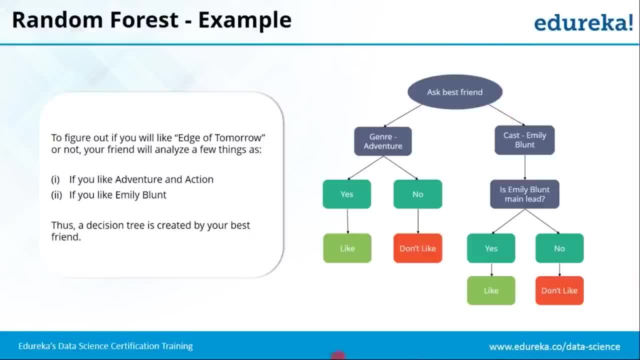 your one decision tree, or you can say your final outcome will be based on just one friend. now, definitely, you're not really convinced. you want to consider the options of your other friends also so that you can make very precise and crisp decision. right, you go out and you approach some other bunch of friends of 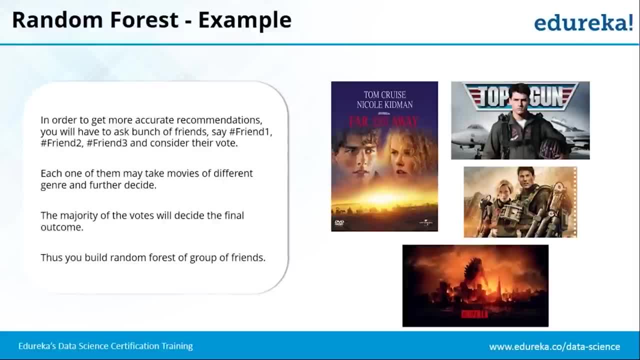 yours. so now, let's say you go to three of your friends and you ask them the same question: whether I would like to watch edge of tomorrow or not. so you go to an approach three of your friends: friend one, friend two and friend three. now you will consider each of theirs, vote and 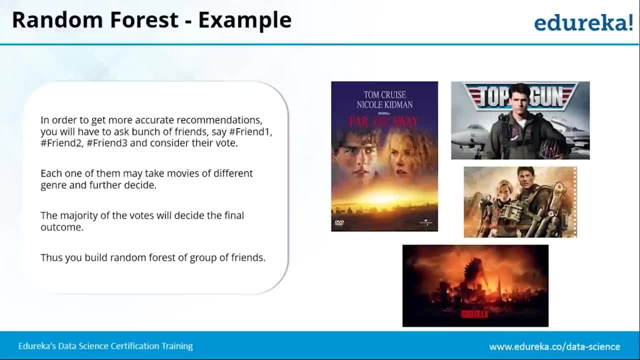 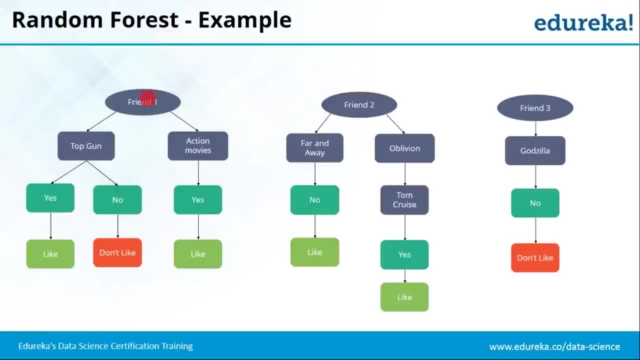 then you will. your decision now will be dependant on the compiled results of all of your three friends right now here. let's say you go to your first friend and you ask him whether you would like to watch edge of tomorrow or not. and your first friend puts you to one question: did you like? 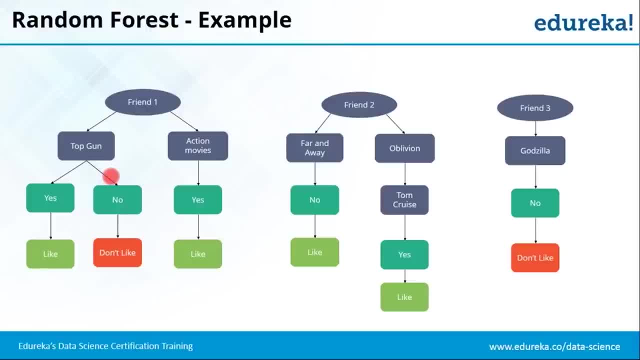 Top Gun and you say, yes, definitely, I did like the movie Top Gun and the probabilities that you would like edge of tomorrow as well, because Top Gun is actually a military action drama, which was so Tom Cruise. so now again, the probability arises that, yes, you will like edge of tomorrow as well, and if you 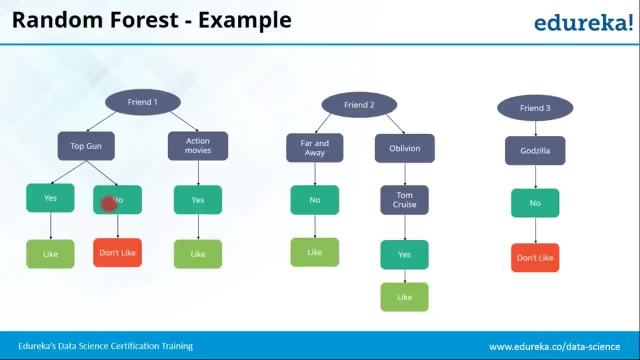 say no, I didn't like Top Gun, then again the chances are that you wouldn't like edge of tomorrow. right, and then another question that he puts you across is that: do you really like to watch action movies? and you say yes, I would love to watch them, then again the chances are that you would like to watch edge of. 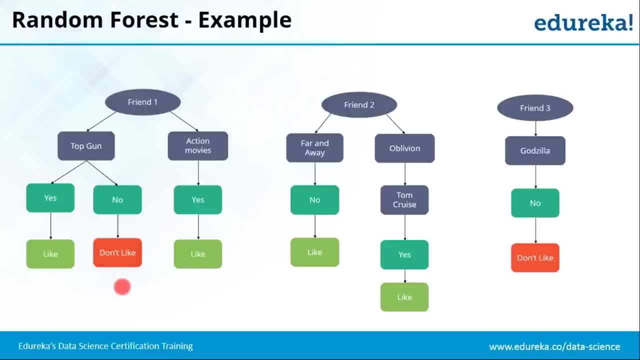 tomorrow. so from your friend one, you can come to one conclusion now here, since the ratio of liking the movie to don't like is actually two is to one. so the final result is actually: you would like edge of tomorrow. now you go to your second friend and you ask the same question. so now your second friend asks: you did you like far and away when we 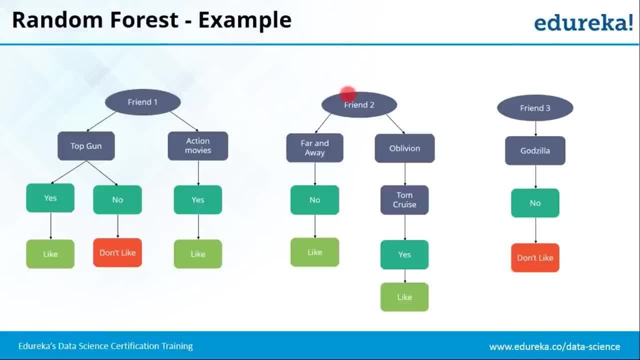 Now you go to your second friend and you ask the same question. So now your second friend asks you, did you like far and away when we went out and the last time when we watched it? and you say, no, I really didn't like far and away. 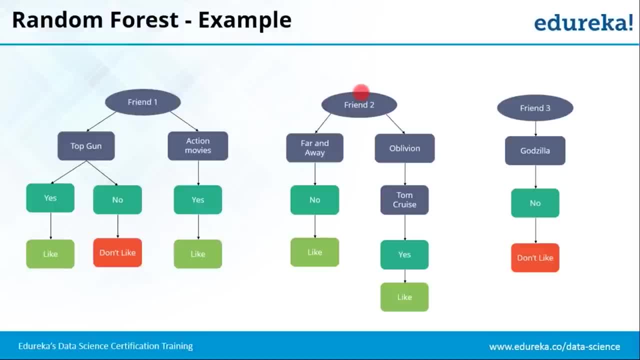 Then you would say: then you are definitely going to like Edge of Tomorrow. Why it is so? because far and away is actually- Most of you might not be knowing it- So far and away is genre of romance and it revolves around a girl and a guy falling in. 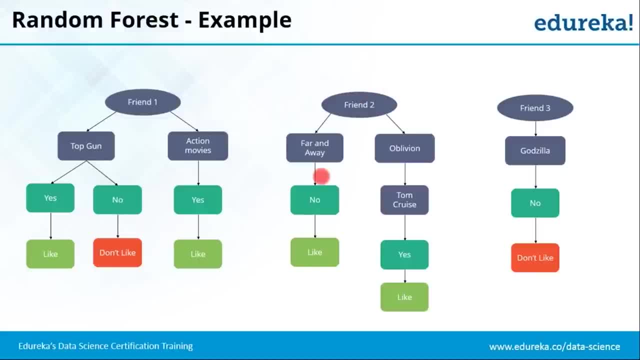 love with each other and so on. So the probability is that you wouldn't like Edge of Tomorrow. So he asked you another question: Did you like Oblivion and do you really like to watch Tom Cruise? and you say yes, and again the probabilities that you would like to watch Edge of Tomorrow. and why? because Oblivion, again, is a 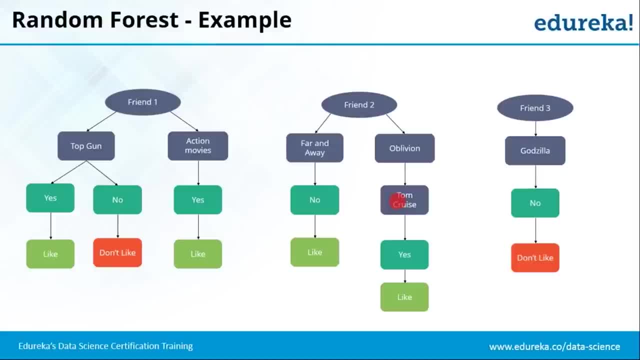 science fiction casting Tom Cruise, full of strange experiences and where Tom Cruise is the savior of the mankind. Well, that is the same kind of plot in Edge of Tomorrow as well. So here it is pure Yes that you would like to watch Edge of Tomorrow. 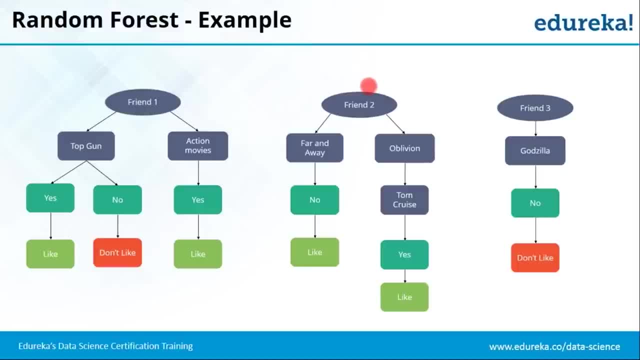 So you get another second decision from your second friend. Are you go to your third friend and ask him? so probably your third friend is not really interesting in having any sort of conversation With you. So it just simply asks you, did you like Godzilla? and you say no, I didn't like Godzilla. 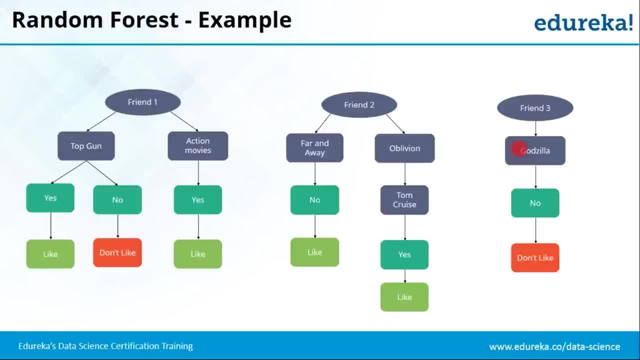 So you say definitely you wouldn't like Edge of Tomorrow. Why so? because Godzilla is also actually a science fiction movie from the Adventure genre. So now you've got three results from three different decision trees from three different friends. Now you compile the results of all those friends and then you make a final call that yes. 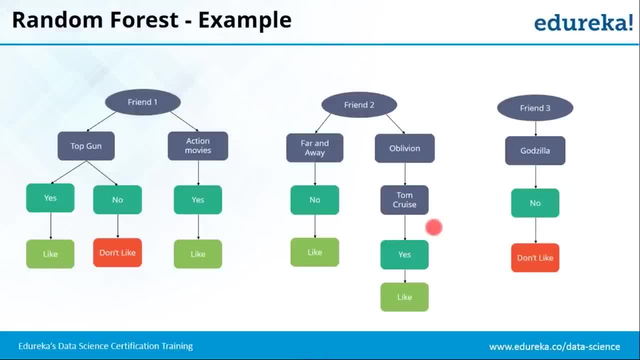 Would you like to watch Edge of Tomorrow Or not? So this is some very real time and very interesting example where you can actually implement random forest into ground reality. Right, any questions? so far, No, that's good, And then we can move forward. 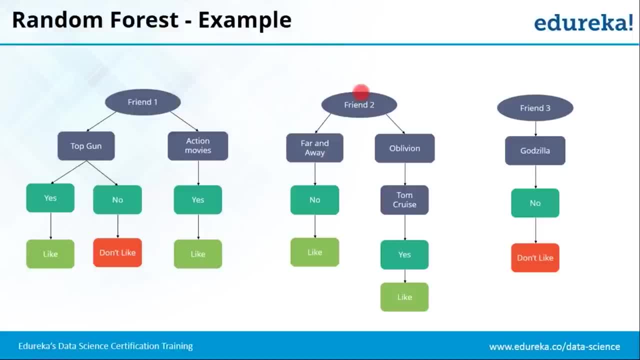 went out and the last time when we watched it and you say, no, i really didn't like far and away, then you would say: then you are definitely going to like edge of tomorrow. why it is so? because far and away is actually- since most of you might not be knowing it- so far and away is genre of romance. 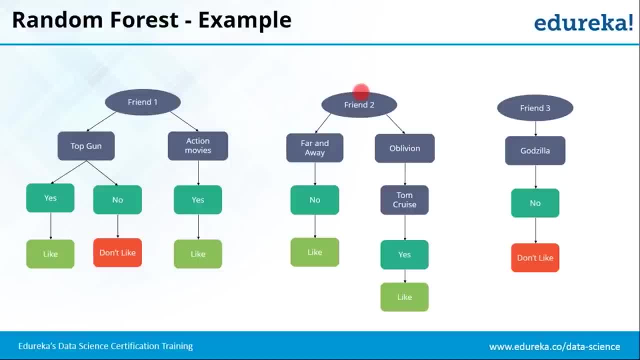 and it revolves around a girl and a guy falling in love with each other and so on. so the probability is that you wouldn't like edge of tomorrow. so he asked you another question: did you like oblivion and do you really like to watch tom cruise? and you say yes and again. 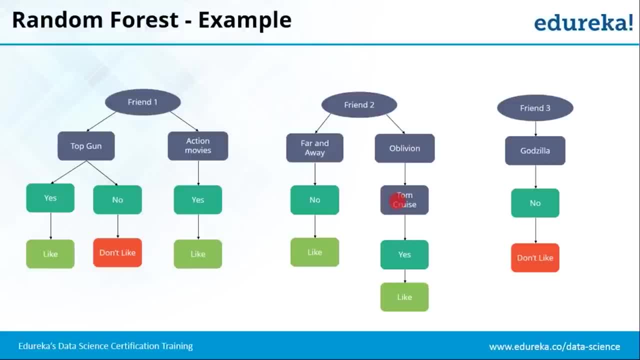 the probability is that you would like to watch edge of tomorrow. why? because oblivion, again, is a science fiction casting tom cruise, full of strange experiences and where tom cruise is the savior of the mankind. well, that is the same kind of plot in edge of tomorrow as well, so here it is pure yes. 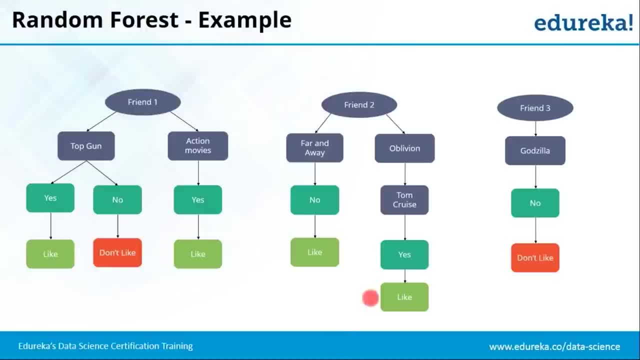 that you would like to watch edge of tomorrow. so you get another second decision from your second friend. now you go to your third friend and ask him. so probably your third friend is not really interested in having any sort of conversation with you, so it just simply asks you, did you like godzilla? and you say no, i didn't like. 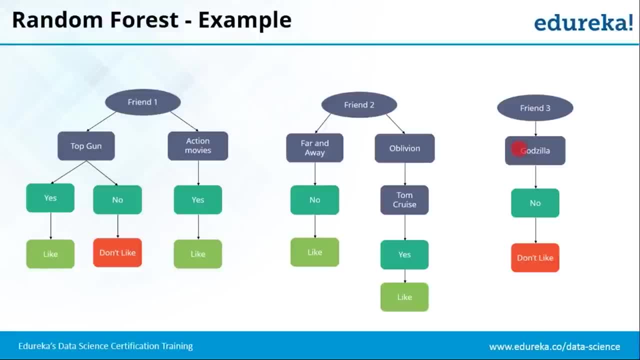 godzilla. so you say, definitely you wouldn't like edge of tomorrow. why so? because godzilla is also actually a science fiction movie from the adventure genre. so now you've got three results from three different decision trees from three different friends. now you compile the results of all those friends and then you make a final call that yes, would you like to watch edge. 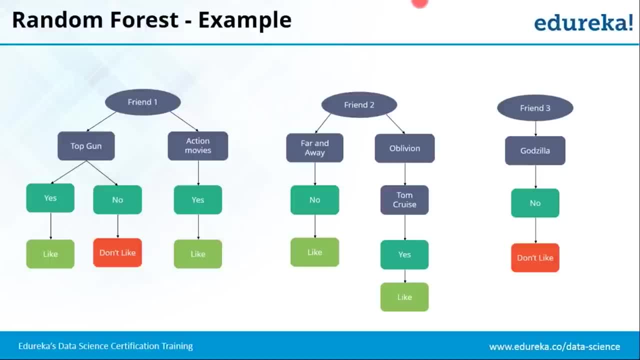 of tomorrow or not. so this is some very real time and very interesting example where you can actually implement random forest into ground reality. right? any questions? so far, no, that's good, and then we can move forward. now let us look at various domains where random forest is actually used. 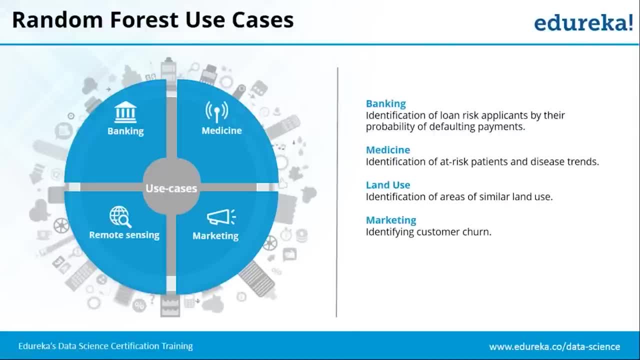 Now let us look at various domains where random forest is actually used. So, because of its diversity, random forest is actually used in various diverse domains like: so beat banking, beat medicine, beat land use, beat marketing- name it, and random forest is there. So in banking, particularly, random forest is being actually used to make it out whether the applicant 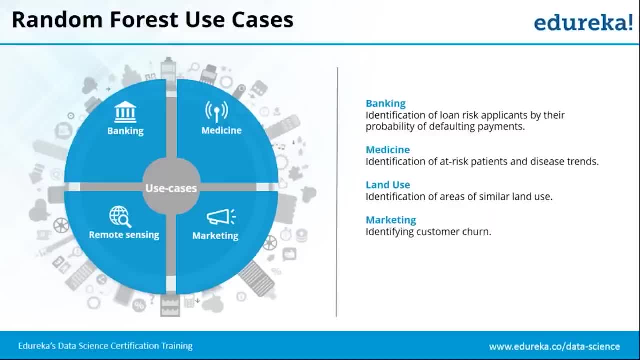 will be a default, a pair, or it will be non-default- a one, so that it can accordingly approve or reject the applications of loan right. So that is how random forest is being used in banking. talking about medicine, random forest Is widely used in medicine field to predict beforehand. 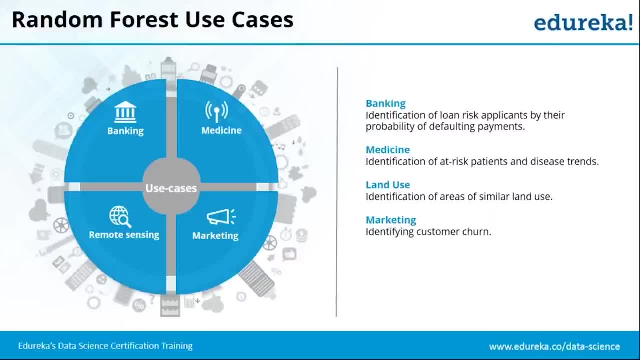 What is the probability if a person will actually have a particular disease or not, right? So it's actually used to look at the various disease Trends. Let's say you want to figure out what is the probability that a person will have diabetes or not. 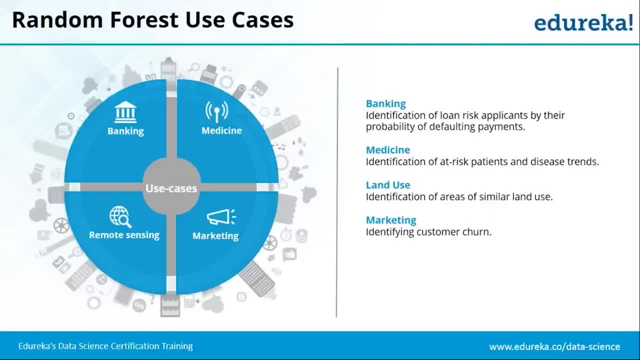 And so what would you do? You'll probably look at the medical history of the patient and then you will see. all right, This has been the glucose concentration. What was the BMI? What was the insulin levels in the patient in the past previous three months? 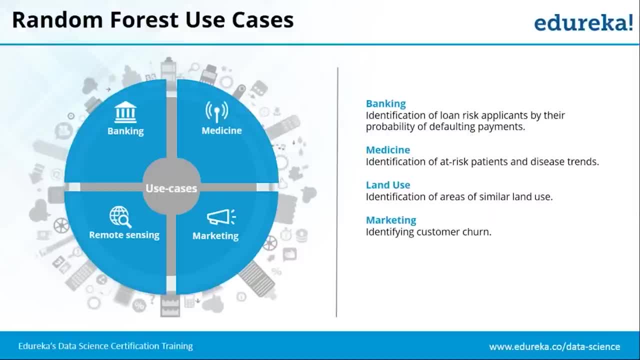 What is the age of this particular person, and you will make different decision trees based on each one of these predicted variables and then you will finally compile the results of all those variables and then you will make a final decision as to whether the person will have diabetes in the near future. 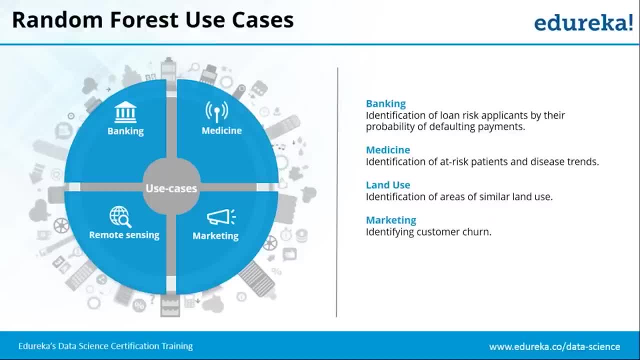 or not. That is how random forest will be used in medicine sector. Now, random forest is also Actually used to find out the land use. for example, I want to set up a particular industry in certain area, So what would I probably look for and look for? 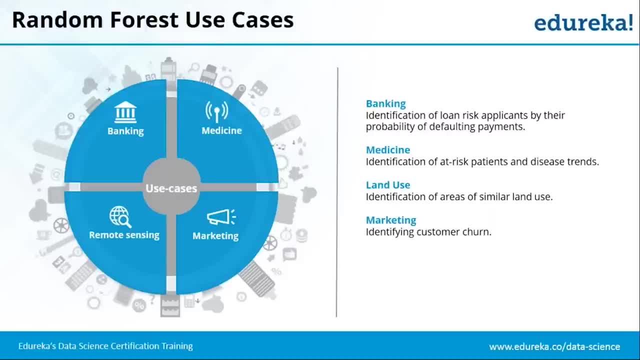 What is the vegetation over there, What is the urban population over there Right, and how much is the distance from the nearest modes of transport, like from the bus station or the railway station? and accordingly, I will split my parameters and I will make decision on each one of these parameters. and finally, 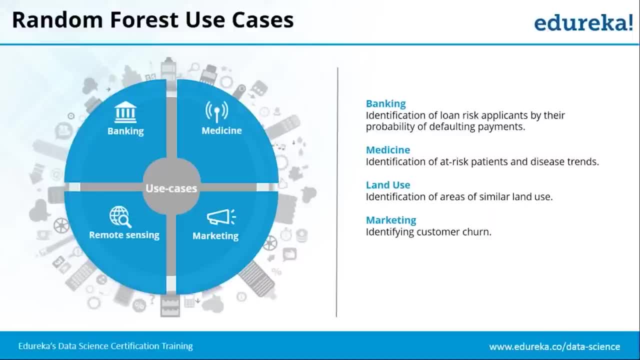 so, because of its diversity, random forest is actually used in various diverse domains. right. so, beat banking, beat medicine, beat land use, beat marketing, name it, and random forest is there. so in banking, particularly random forest is being actually used to make it out whether the applicant will be a defaulter pair or it will be non-default one, so that it can accordingly 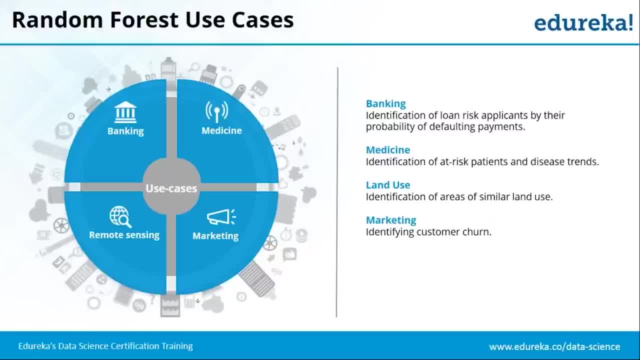 approve or reject the application of random forest loan. right, so that is how random forest is being used in banking. talking about medicine, a random forest is widely used in medicine field to predict beforehand what is the probability if a person will actually have a particular disease or not. right, so it's actually used to look at the various disease trends. let's say: 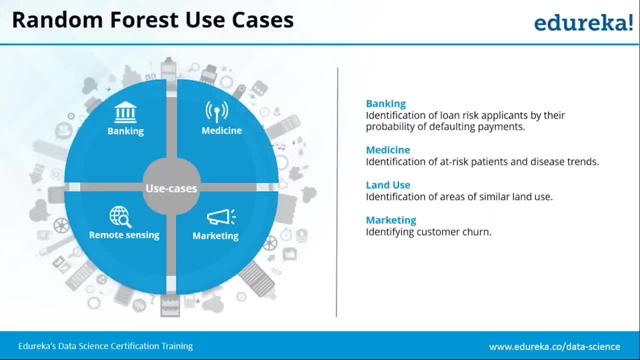 you want to figure out what is the probability that a person will have diabetes or not, and so what would you do? you'll probably look at the medical history of the patient and then you will see. all right, this has been the glucose concentration. what was the BMI? what was the insulin levels in the 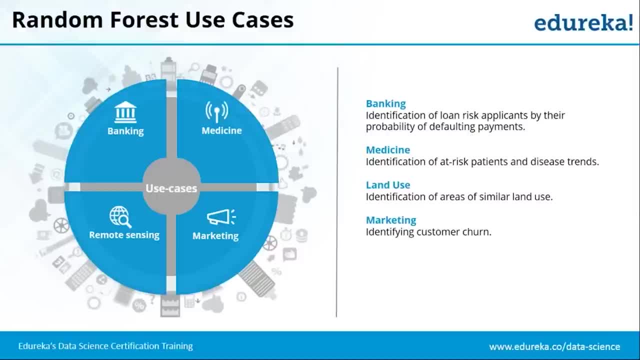 patient in the past previous three months, what is the age of this particular person? and you will make different decision trees based on each one of these predicted variables and then you will finally compile the results of all those variables and then you will make a final decision as to. 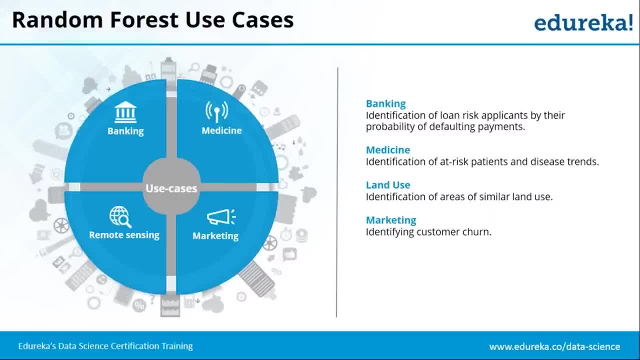 whether the person will have diabetes in the near future or not. that is how random forest will be used in medicine sector. now, random forest is also actually used to find out the land use. for example, I want to set up a particular industry in certain area, so what would I probably look for? I look, 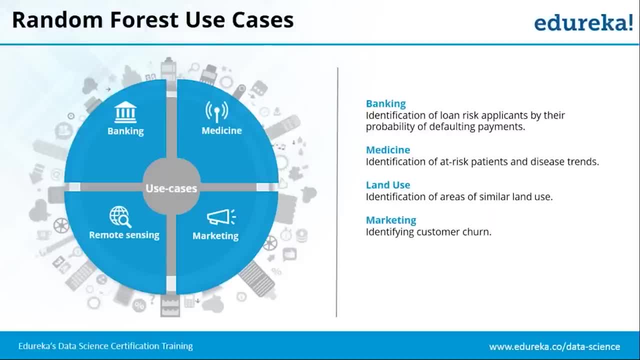 for what is the vegetation over there, what is the urban population over there right, and how much is the distance from the nearest modes of transport, like from the bus station or the railway station? and accordingly, I will split my parameters and I will make decision on each one of these parameters and finally I'll compile my decision of all these. 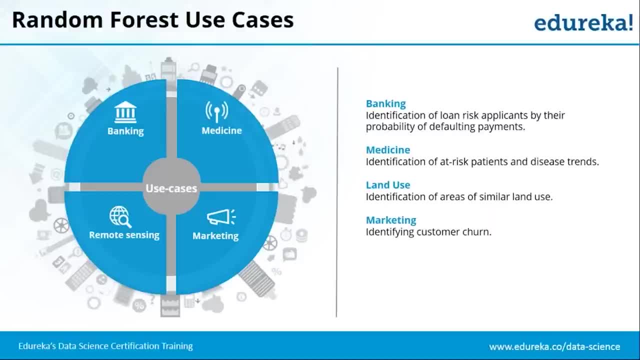 I'll compile my decision of all these parameters and that will be my final outcome. So that is how I'm finally going to predict whether I should put my industry at this particular location or not, right? So these three examples have actually been of majorly around classification problem, because we are trying to classify. 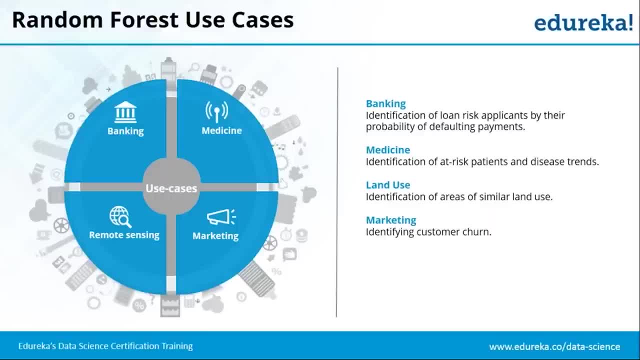 whether or not, with actually trying to answer this question, whether or not right now, let's move forward and look how marketing Is revolving around random forest. So particularly in marketing we try to identify the customer churn. So this is particularly the regression kind of problem. 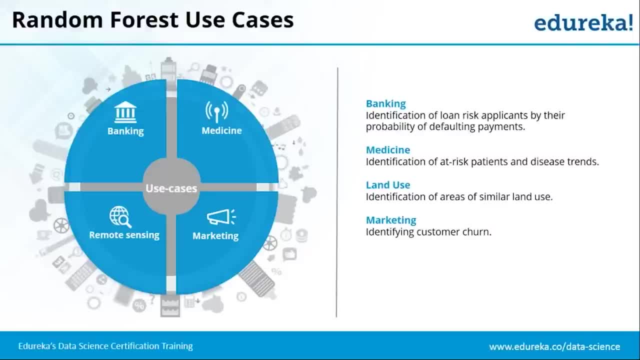 right Now how let's see so customer churn is nothing, but actually the number of people which are actually, or the number of customers who are losing out. So we're going out of your market. Now you want to identify what will be your customer churn in near future. 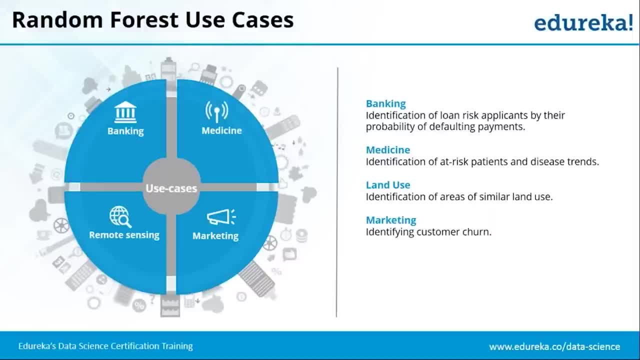 So you'll. most of the e-commerce Industries are actually using this, like Amazon, Flipkart, Etc. So they particularly look at your each behavior as to what has been your past history, What has been your purchasing history, What do you like based on your activity around certain things, around certain ads, around certain discounts or around certain kind of materials? 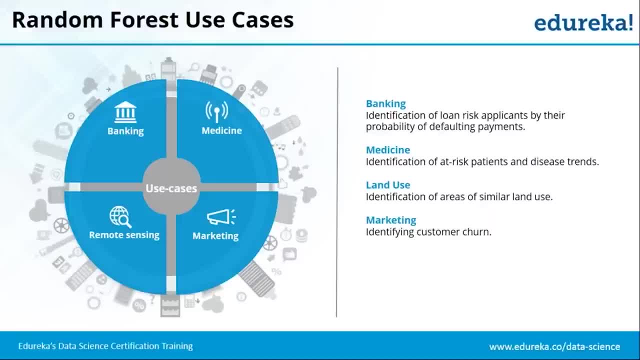 right. If you like a particular top, your activity will be more around that particular top. So that is how they track each and every particular move of Yours, and then they try to predict whether you will be moving out or not. So that is how they identify the customer churn. 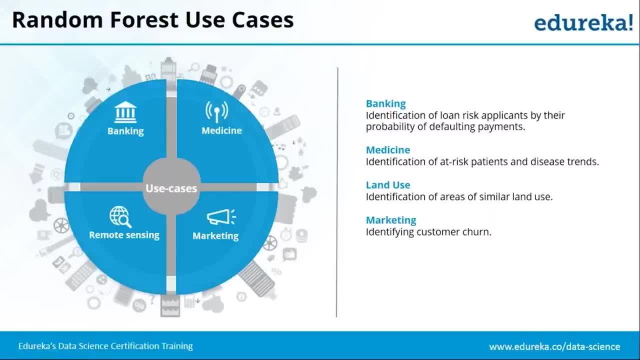 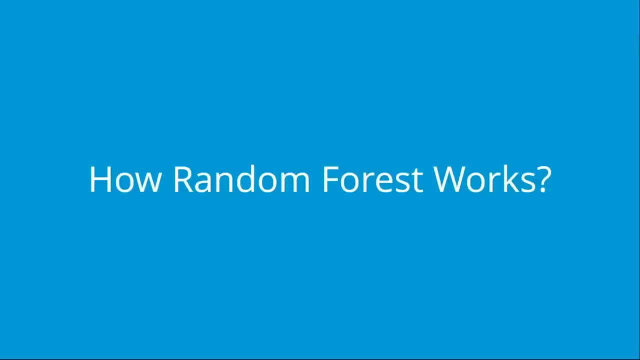 So these all are various domains where random forest is used, and this is not the only list, So there are numerous other examples which actually are using random forests. that makes it so special actually. Now let's move forward and see how random forest actually works. 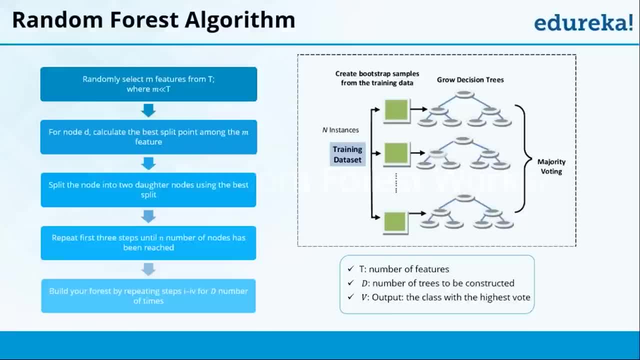 right. So let us start with the random For this algorithm first. Let's just see it step by step as to how random forest algorithm works. So the first step is to actually select certain M features from T where M is less than T. 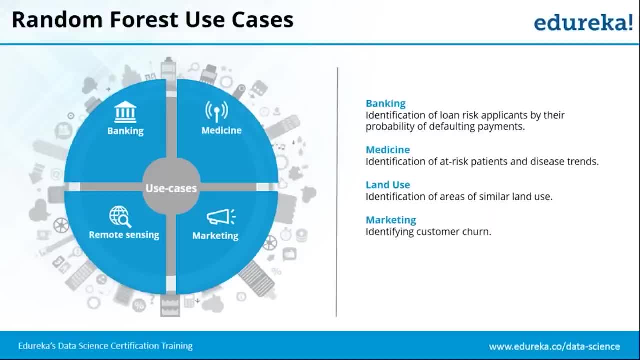 parameters and that will be my final outcome. so that is how I am finally going to predict whether I should put my industry at this particular location or not, right? so these three examples have actually been of majorly around classification problem, because we are trying to classify whether or not. 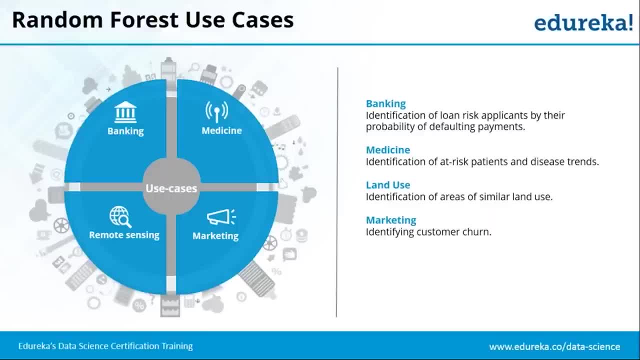 we're actually trying to answer this question, whether or not right now. let's move forward and look how marketing is revolving around random forest. so particularly in marketing we try to identify the customer churn. so this is particularly the regression kind of problem right now. how let's see so 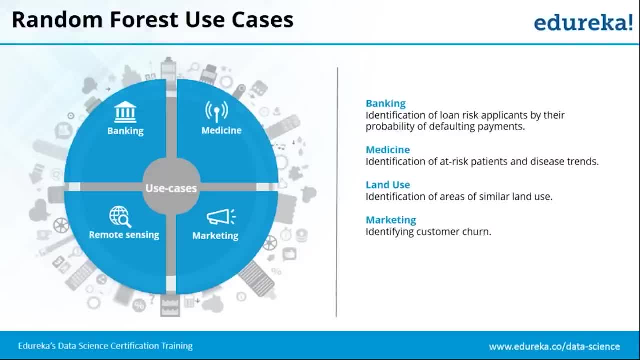 customer churn is nothing, but actually the number of people which are actually, or the number of customers who are losing out. so we're going out of your market. now you want to identify what will be your customer churn in near future. so most of the e-commerce industries are actually using this like. 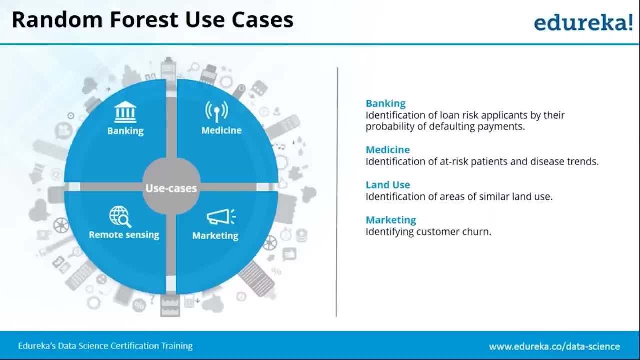 Amazon, Flipkart, etc. so they particularly look at your each behavior as to what has been your past history, what has been your purchasing history, what do you like based on your activity around certain things, around certain ads, around certain discounts or around certain kind of materials? right, if you like your. 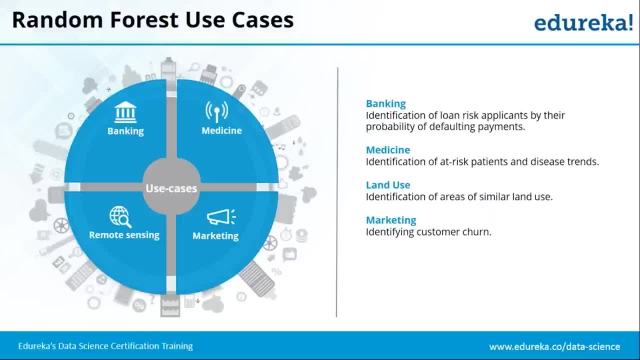 particular top, your activity will be more around that particular top. so that is how they track each and every particular move of yours, and then they try to predict whether you will be moving out or not. so that is how they identify the customer churn. so these all are various domains where random forest. 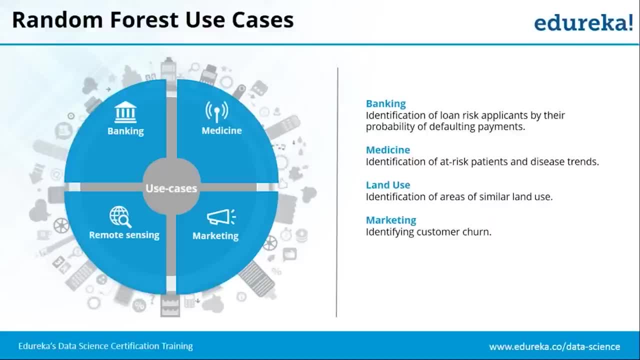 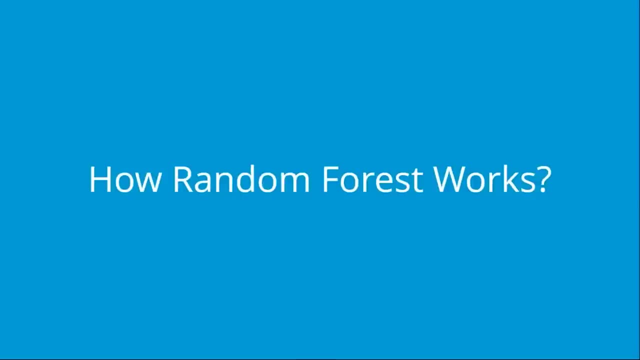 is used, and this is not the only list, so there are numerous other examples which actually are using random forests. that makes it so special, actually. now let's move forward and see how random forest actually works, right, so let us start with the random forest algorithm first. let's just see it. 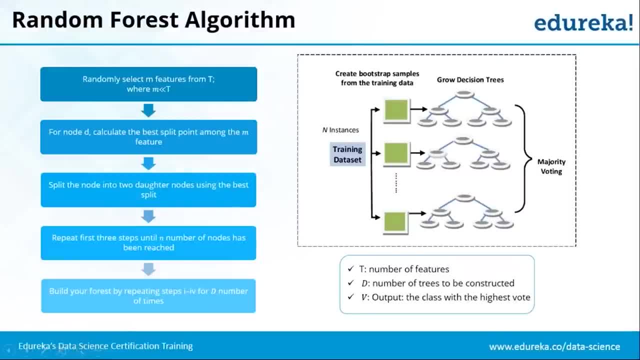 step-by-step as to how random forest algorithm works. so the first step is to actually select certain M features from T where M is less than T. so here T is the total number of the predicted variables that you have in your data set, and out of those total predicted variables you will select some. 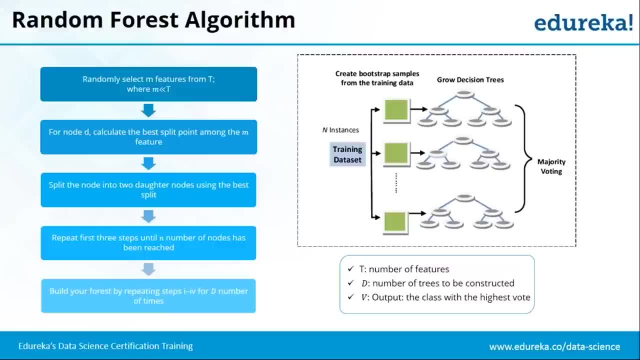 So here, T is the total number of the predictor variables that you have in your data set, and out of those total predictor variables You will select some randomly, some few features out of those. Now, why we are actually selecting a few features only? The reason is that if you will select all the predictor variables or the total predictor variables, 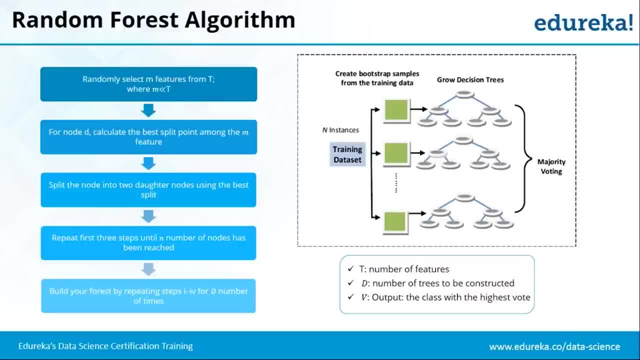 then each of your decision tree will be same. So your model is not actually learning something new, It is learning the same previous thing, because all those decision trees will be similar, right? If you actually split your predicted variables and you select randomly a few predicted variables only? 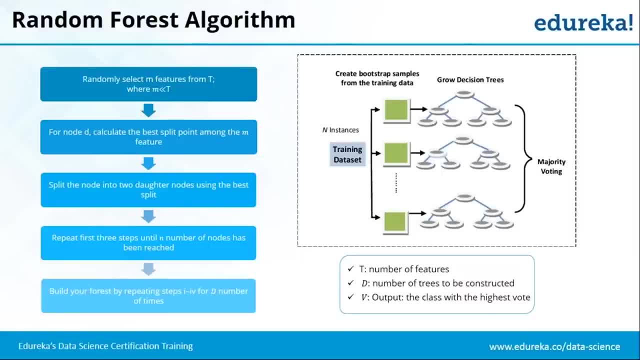 let's say there are 14 total number of variables and out of those you randomly pick just three, right? So every time you will get a new decision tree, So there will be variety, right? So the classification model will be actually much more intelligent than the previous one. 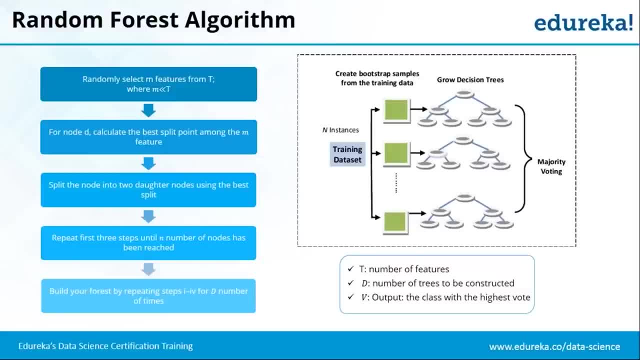 Now it has got varied experiences, So definitely it will make different decisions each time and then, when you will compile all those different decisions, it will be a new, more accurate and efficient result, Right? So the first important step is to select certain. 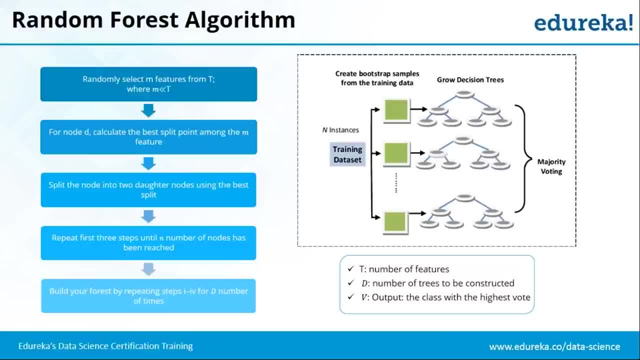 Number of features out of all the features. Now let's move on to the second step. Let's say, for any node D. Now the first step is to calculate the best split at that point. So you know that decision tree, how decision tree is actually implemented. 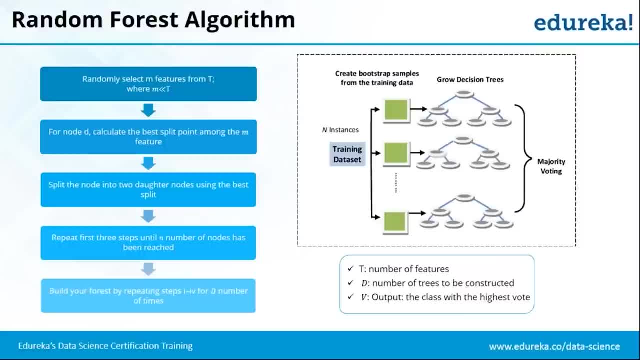 So you pick up the most significant variable, right, And then you will split that particular node into further child nodes. That is how the split takes place, right. So you will do it for M number of variables That you've selected. Let's say you have selected three. 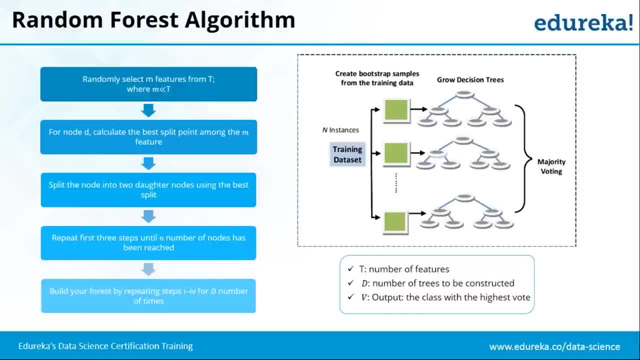 So you will implement the split at all those three nodes in one particular decision tree, right? The third step is split of the node into two daughter nodes. So now you can split your root node into as many nodes as you want to, but here will split our node into two daughter nodes as to this or that. 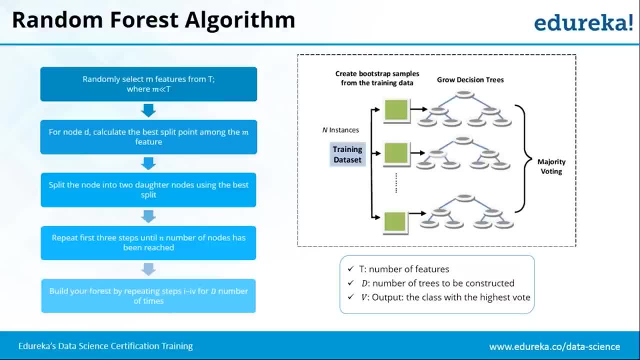 randomly some few features out of those. now why we are actually selecting a few features only? the reason is that if you will select all the predictive variables, or the total predicted variables, then each of your decision tree will be same. so your model is not actually learning something new, it is learning the same. 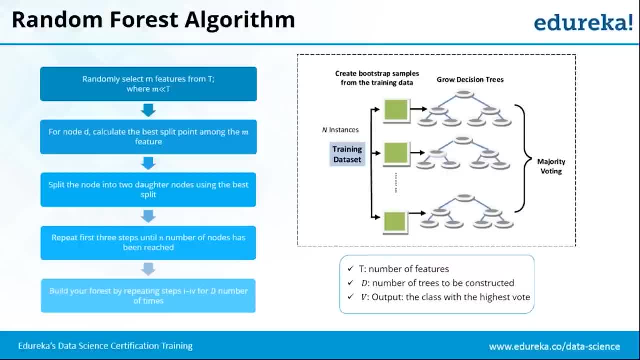 previous thing, because all those decision trees will be similar right now if you actually split your predicted variables and you select randomly a few predicted variables only. let's say there are 14 total number of variables and out of those you'll randomly pick just three, right? so every time you will get a new. 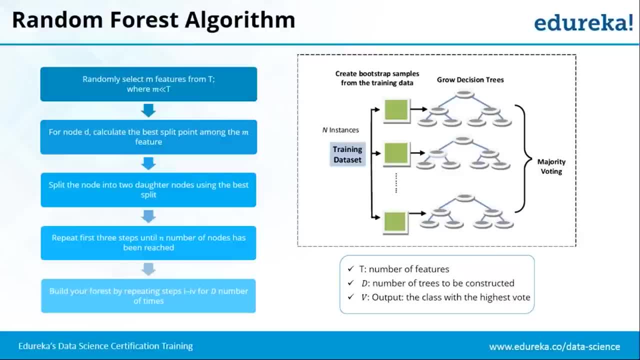 decision tree, so there will be variety, right. so the classification model will be actually much more intelligent than the previous one now it has got varied experiences, so definitely it will make different decisions each time and then, when you will compile all those different decisions, it will be a new, more accurate and efficient result, right? so the first important step is to 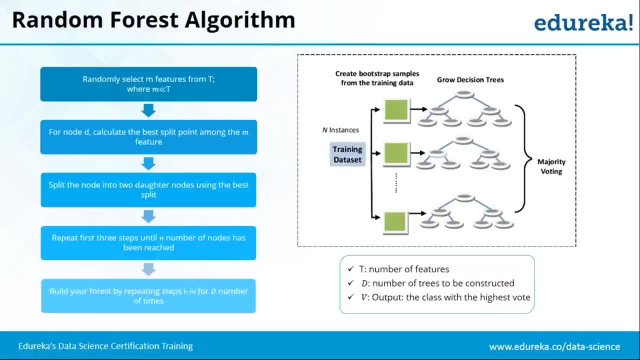 select certain number of features out of all the features. now let's move on to the second step. let's say, for any node D, now the first step is to calculate the best split at that point. so you know that decision tree, how decision tree is actually implemented. so you pick up the most significant variable right and then 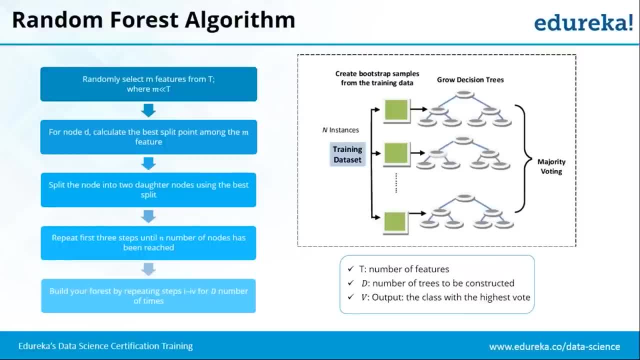 you will split that particular node into further child nodes. that is how the split takes place, right? so you will do it for M number of variables that you've selected. let's say you have selected three, so you will implement the split at all those three nodes in one particular decision tree, right? the third step is split of the. 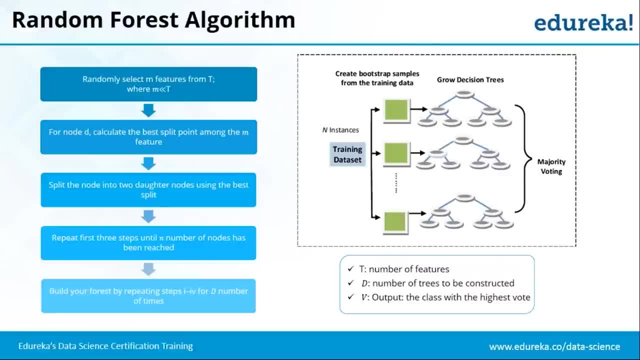 node into two daughter nodes. so now you can split your root node into as many nodes as you want to, but here we'll split our node into two daughter nodes as to this or that, so it will be an answer in terms of this or that right. our fourth step will 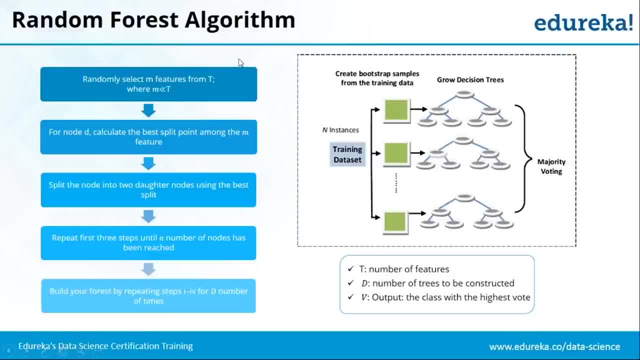 So it will be an answer in terms of this or that, right. Our fourth step will be to repeat all these three steps That we've done previously, and will repeat all this splitting until we have reached all the N number of nodes, right. 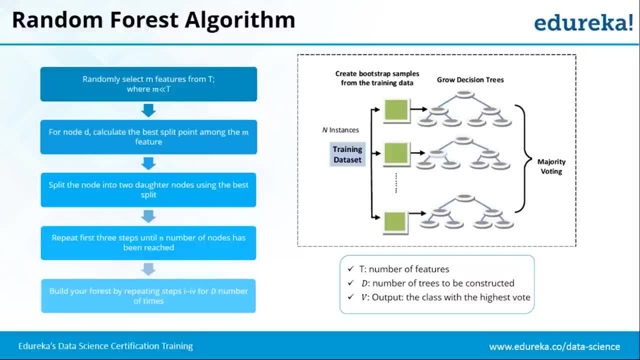 So we need to repeat until we have reached till the leaf nodes of a decision tree. That is how we will do it right now. After these four steps, we will have our one decision tree, but random forest is actually about multiple decision trees. 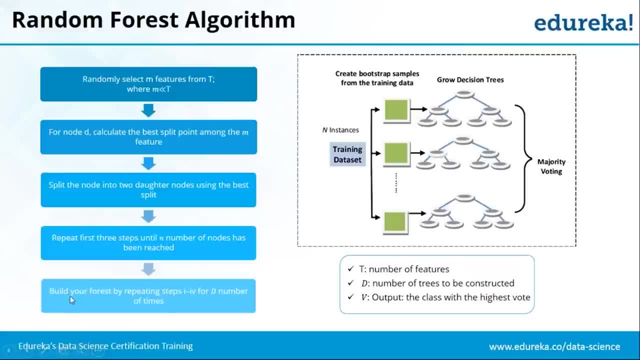 So here our fifth step will come into the picture, which will actually repeat all these previous steps for D number of times. Now here, D is the D number of decision trees. Let's say I want to implement five decision trees, So my first step will be to implement all the previous steps five times. 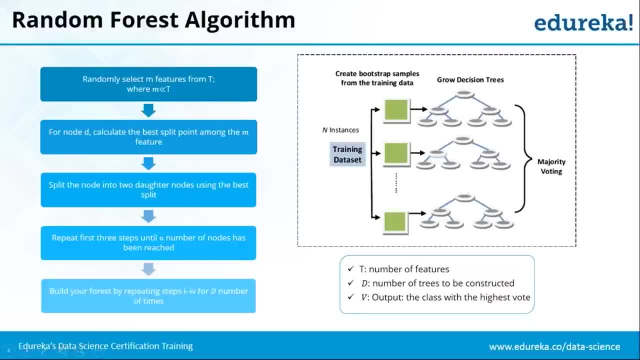 So the head, the iteration is for five number of times right Now, once I have created these five decision trees, still, my task is not complete yet. Now my final task will be to compile the results of all these five different decision trees and I will make a call in the majority voting right here. 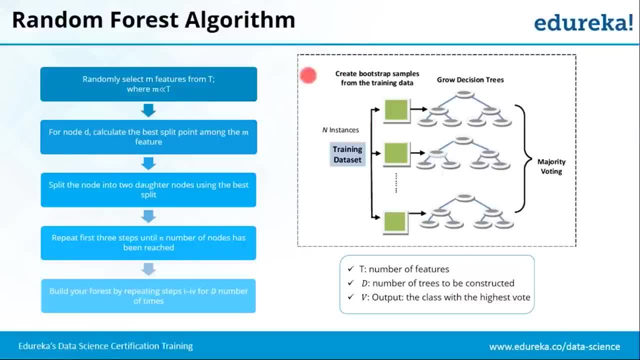 As you can see in this picture, I had N different instances, Then I created N different decision trees And finally I will compile the result of all these N different decision trees and I'll take my call on the majority voting right. So, whatever my majority vote says, that will be my final result. 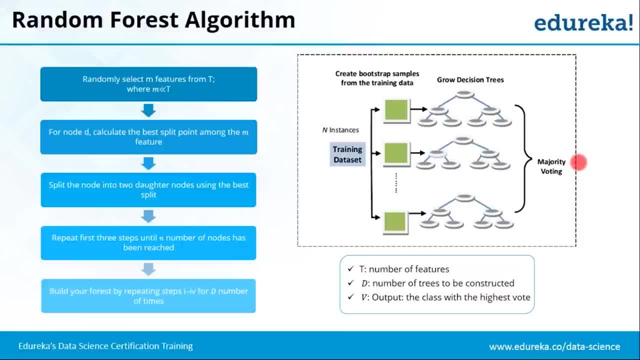 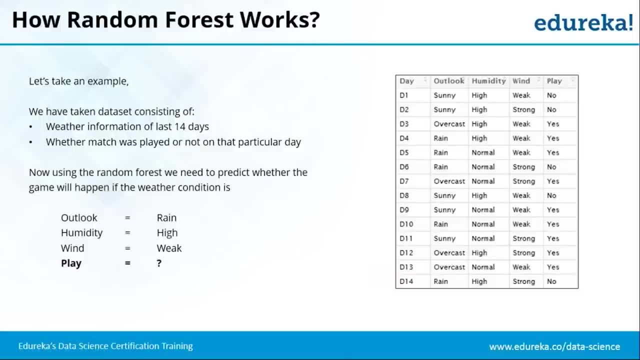 So this is basically an overview of the random forest algorithm. So this is basically an overview of the random forest algorithm. So this is basically an overview of the random forest algorithm- How it actually works. Let's just have a look at this example to get much better understanding of what we have learned. 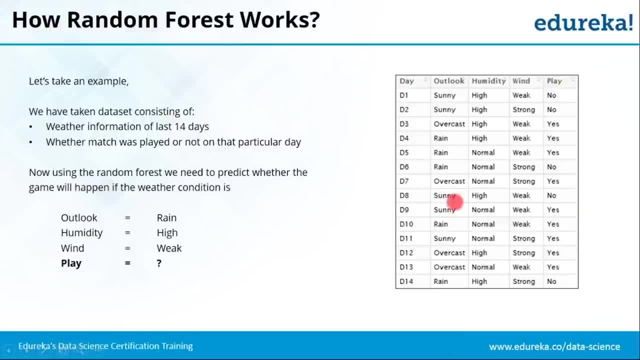 So let's say I have this data set which consists of four different instances, right? So basically, it consists of the weather information of previous 14 days, right from D1 till D14, and this basically outlook humidity and when. this basically gives me the weather condition of those 14 days. 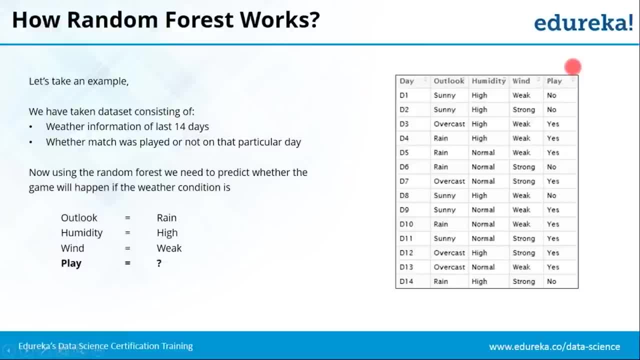 And finally, I have play, which is my task- Target variable where the match did take place on that particular day or not. right Now, my main goal is to find out whether the match will actually take place If I have following these weather conditions with me on any particular day. 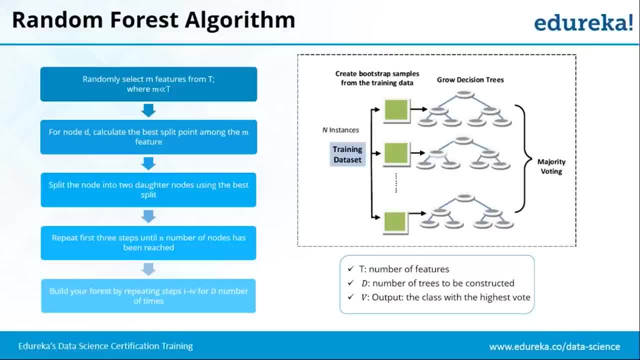 be to repeat all these three steps that we've done previously. and we'll repeat all this splitting until we have reached all the N number of nodes, right. so we need to repeat until we have reached till the leaf nodes of a decision tree. that is how we will do it right now. after these four steps, we will have our 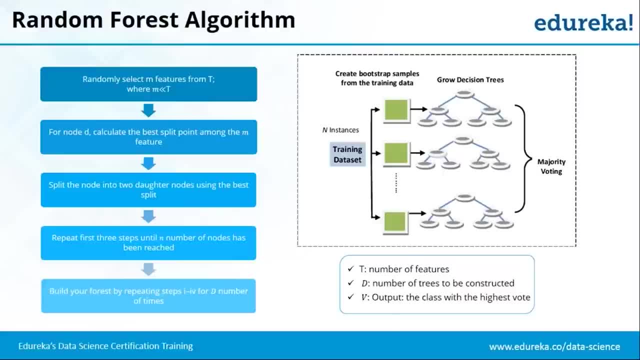 one decision tree, but random forest is actually about multiple decision trees. so here our fifth step will come into the picture, which will actually repeat all these previous steps for D number of times. now here, D is the D number of decision trees. let's say I want to. 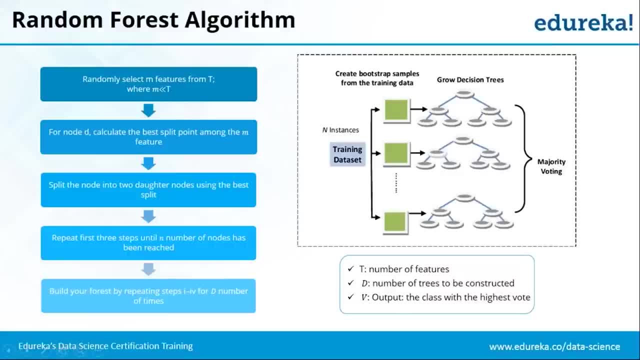 implement five decision trees. so my first step will be to implement all the previous steps five times. so here the iteration is for five number of times. right now, once I have created these five decision trees, still my task is not complete yet. now my final task will be to compile the results of 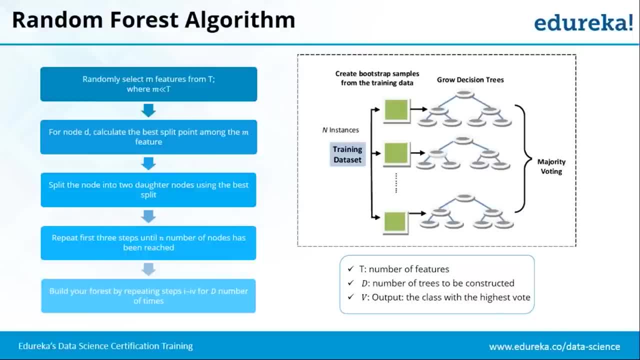 all these five different decision trees and I will make a call in the majority voting right here. as you can see in this picture, I had N different instances, then I created N different decision trees and, finally, I will compile the result of all these N different decision trees and I will take my call on the majority voting. 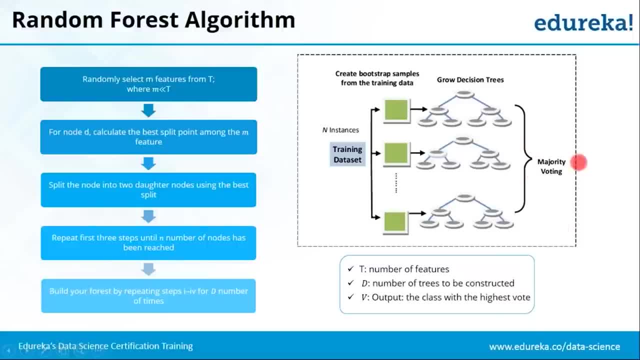 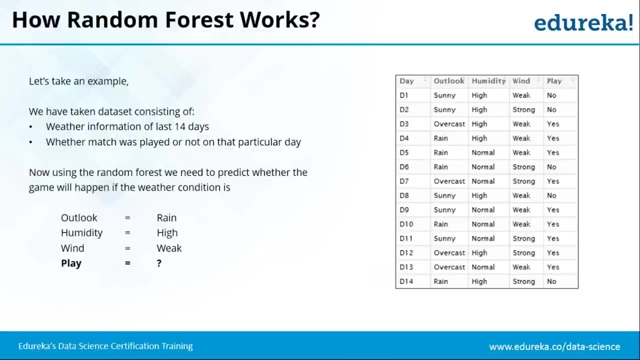 right. so whatever my majority vote says, that will be my final result. so this is basically an overview of the random forest algorithm- how it actually works. let's just have a look at this example to get much better understanding of what we have learnt. so let's say I 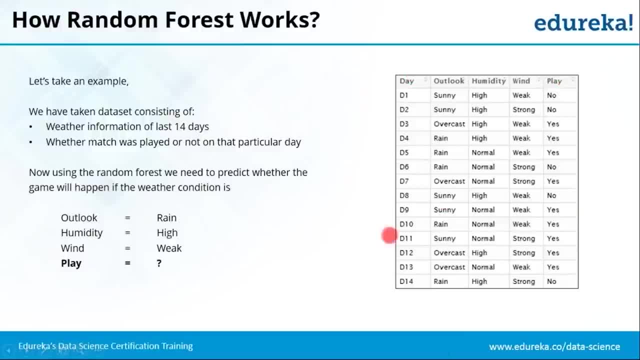 have this data set which consists of four different instances, right? so basically it consists of the weather information of previous 14 days, right from D 1 till D 14, and this basically outlook: humidity and wind. this basically gives me the weather condition of those 14 days. and finally, I have play, which is 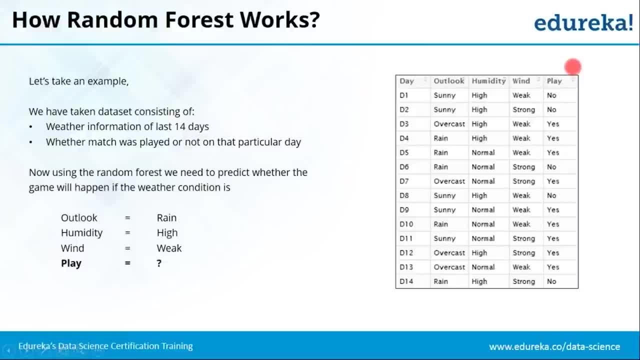 my target variable whether match did take place on that particular day or not. right now, my main goal is to find out whether the match will actually take place if I have following these, whether conditions with me on any particular day, let's say, the outlook is rainy that day and 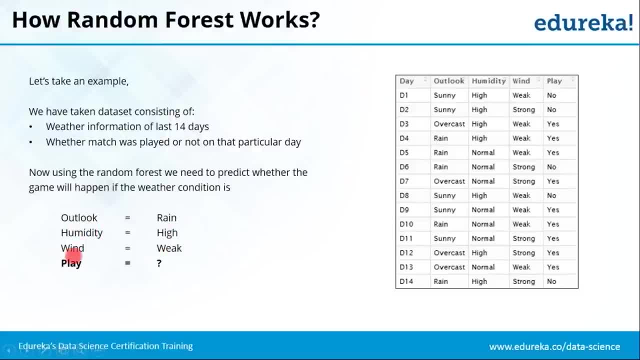 let's say, the outlook is rainy that day and humidity is high and the wind is very weak. So now I need to predict whether I will be able to play the match that day or not. All right, So this is a problem statement. fine. 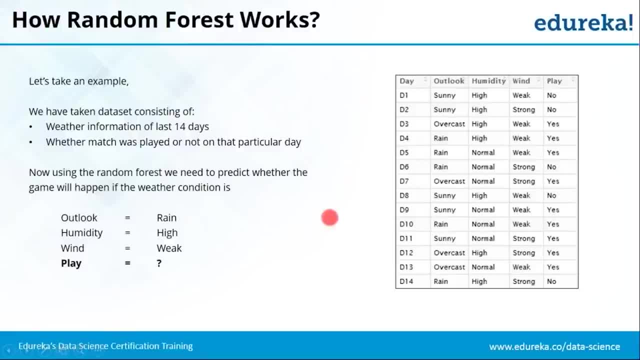 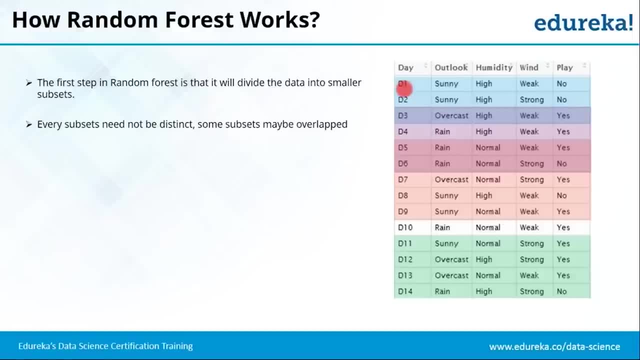 Now let's see how random forest Is used in this to sort it out. Now here, The first step is to actually split my entire data set into subsets. here I have split my entire 14 variables into further smaller subsets, right? 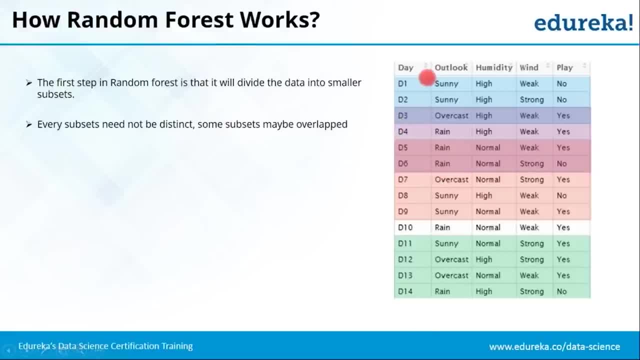 Now these subsets may or may not overlap. like there is certain overlapping between D1 till D3 and D3 till D6. fine, So there is an overlapping of D3. So it might happen that there might be overlapping, So you need not really worry. 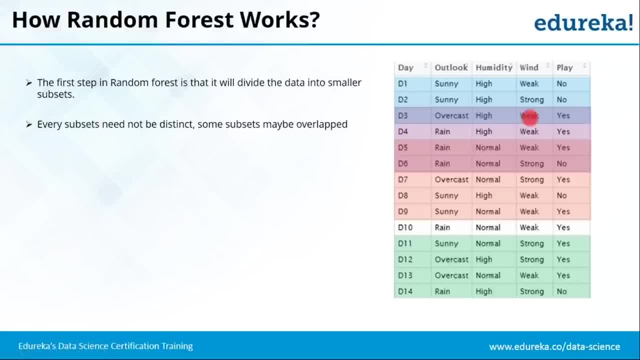 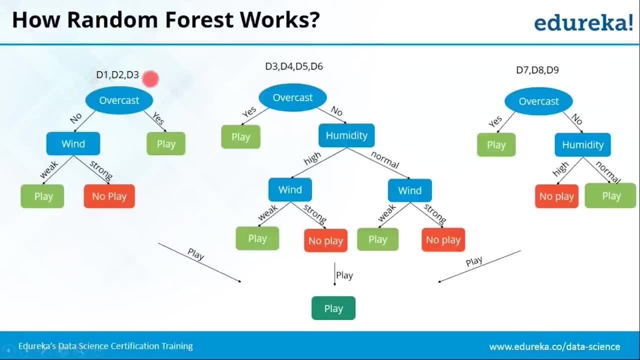 About the overlapping, but you have to make sure that all those subsets are actually different, right? So here I have taken three different subsets. My first subset consists of D1 till D3.. My second subset consists of D3 till D6, and method subset consists of D7 till D. now 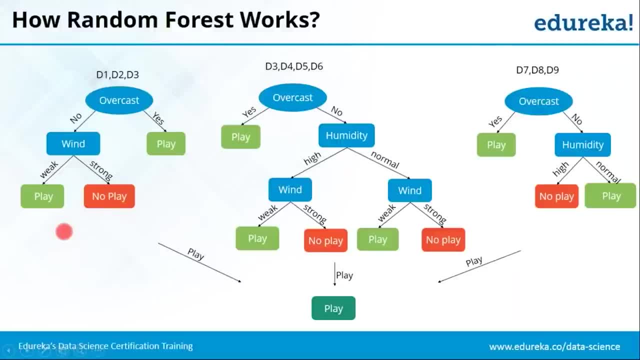 Now I will first be focusing on my first subset Now here. Let's say that particular day The outlook was overcast. fine, If yes, it was overcast, Then the probability is that the match will be overcast. Is that the match will take place? 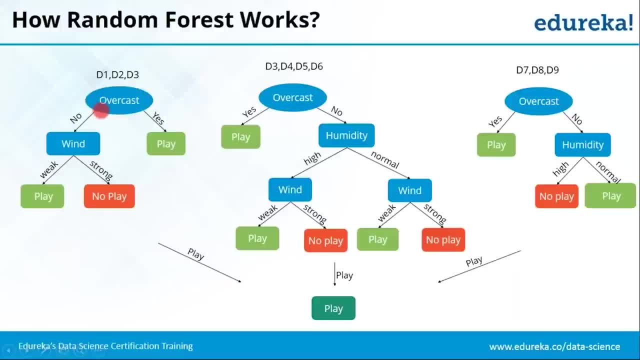 So overcast is basically when your weather is too cloudy. So if that is the condition, then definitely the match will take place. And let's say it wasn't overcast. Then you will consider the second most probable option, That will be the wind, and you will make your decision based on this. 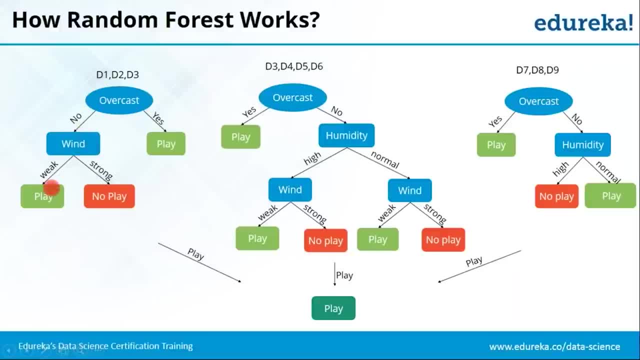 Now whether wind was weak or strong. if it was weak, then you will definitely go out and play the match, else you would not. So now the final outcome out of this Isn't tree will be play, because here the ratio between the play and no play is 2 is to 1.. 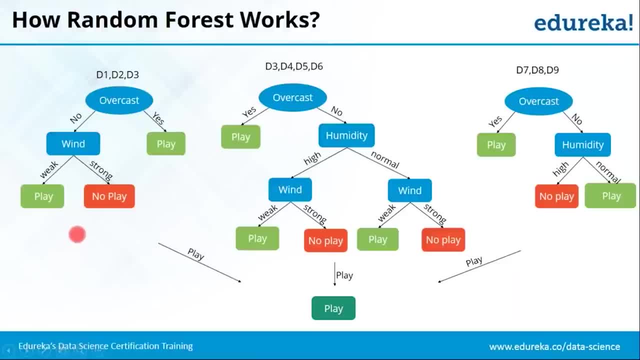 So we get to a certain decision from a first decision tree. Now let us look at the second subset Now, since second subset has different number of variables. So that is why this decision tree is absolutely different from what we saw in our first subset. 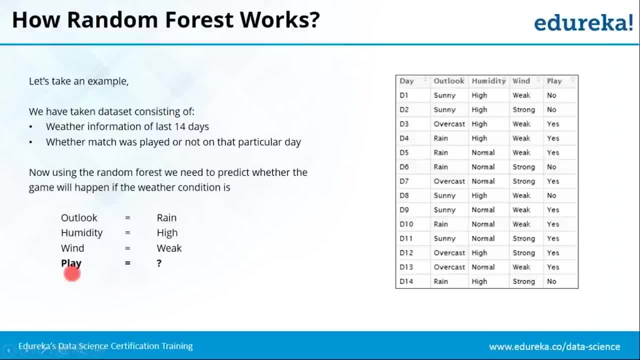 here is basically relative- the weather conditions that I have followed for that 5 days- and humidity is high and the wind is very weak. so now i need to predict whether i will be able to play the match that day or not. all right, so this is a problem statement. fine, now let's see how random 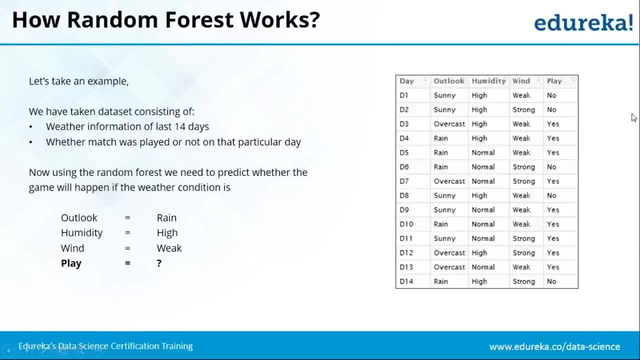 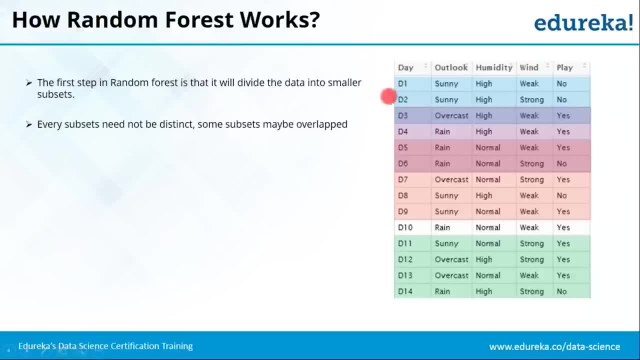 forest is used in this to sort it out now. here the first step is to actually split my entire data set into subsets. here i have split my entire 14 variables into further smaller subsets. right now these subsets may or may not overlap. like there is certain overlapping between d1 till d3. 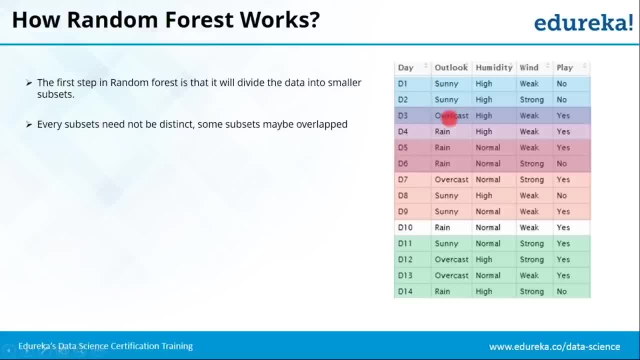 and d3 till d6, right? so there is an overlapping of d3. so it might happen that there might be overlapping. so you need not really worry about the overlapping, but you have to make sure that all those subsets are actually different, right? so here i have taken three different subsets. 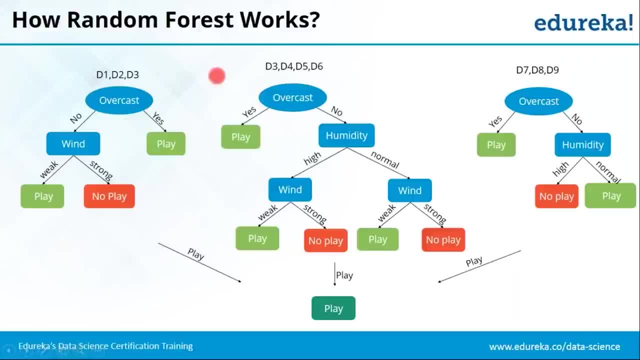 my first subset consists of d1 till d3. my second subset consists of d3 till d6, and my third subset consists of d3 till d6, and my third subset consists of d3 till d6, and my third subset consists of consists of D7 till D now. now I will first be focusing on my first subset now. 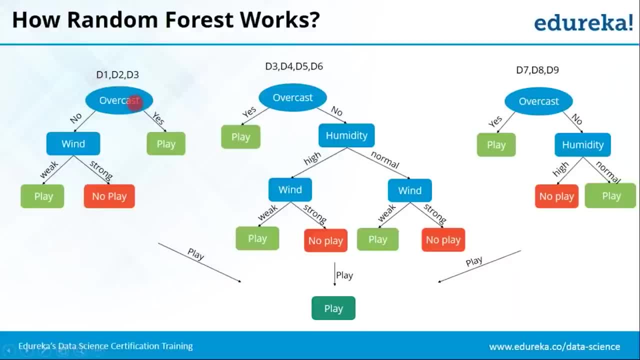 here. let's say that particular day the outlook was overcast, fine, if yes, it was overcast, then the probability is that the match will take place. so overcast is basically when your weather is too cloudy. so if that is the condition, then definitely the match will take place. and let's say it wasn't overcast, then you. 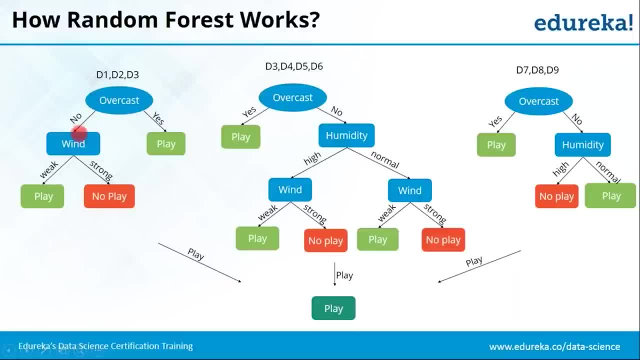 will consider the second most probable option, that will be the wind, and you will make a decision based on this now, whether wind was weak or strong. if it was weak, then you will definitely go out and play the match, else you would not. so now the final outcome out of this decision tree will be play, because here 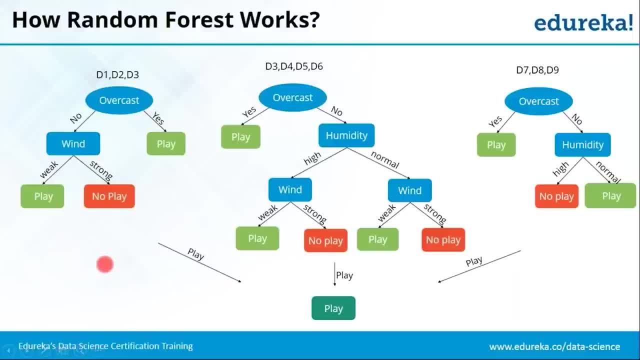 the ratio between the play and no play is 2 is to 1, so we get to a certain decision from a first decision tree. now let us look at the second subset now, since second subset has different number of variables. so that is why this decision tree is absolutely different from what we saw in our first subset. so 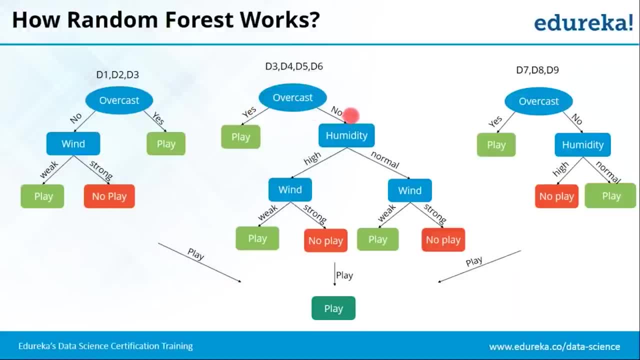 let's say, if it was overcast, then you will play the match. if it isn't the overcast, then you will look out for humidity. now, further, it will get split into two, whether it was high or normal. now we will take the first case. if the humidity was high and wind was weak, then you will play the match. 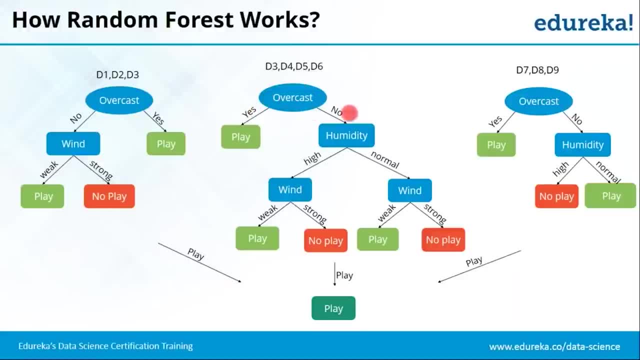 So let's say, if it was overcast then you will play the match. If it isn't the overcast, then you would go and look out for humidity. now, further, It will get split into two, whether it was high or normal. Now we'll take the first case: if the humidity was high and wind was weak. 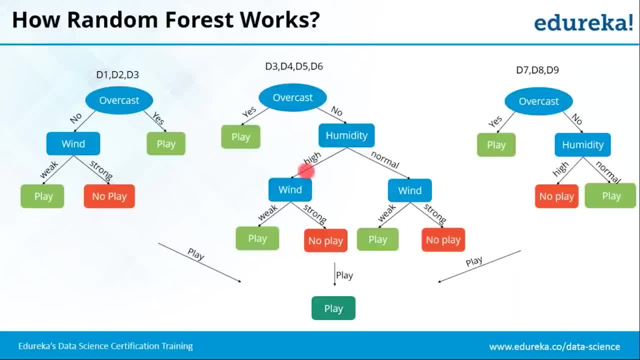 then you will play the match. else, if humidity was high but wind was too strong, then you would not go out and play the match right now. Let us look at the second daughter node of humidity. If the humidity was normal and the wind was weak, 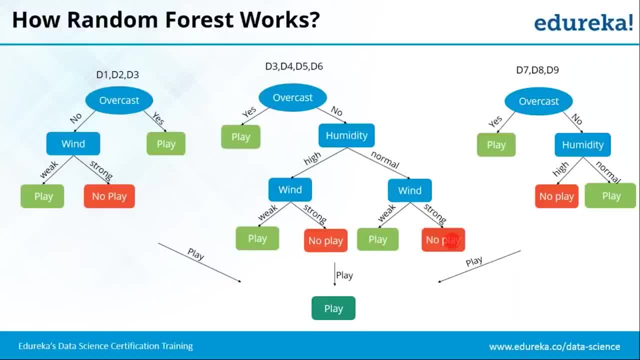 then you will definitely go out and play the match as you want: Go out and play the match. So here, if you look at the final result, then the ratio of plays to no play is 3 is to 2.. Then again, the final outcome is actually play. 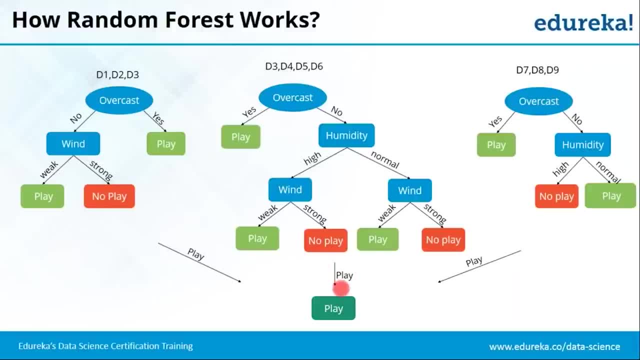 right. So from second subset we get the final decision of play. Now let us look at our third subset, which consists of D7 till D9. here, If again the overcast is yes, then you will play match, else you will go and check out for humidity. 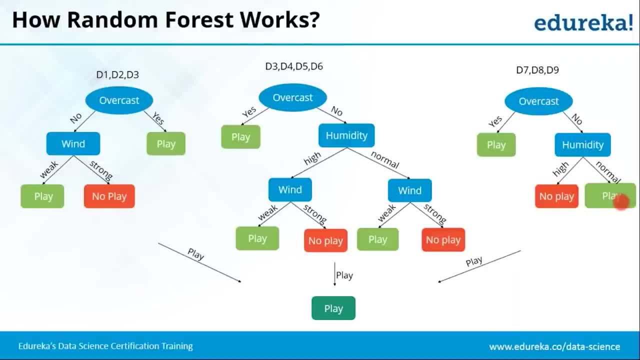 And if the humidity is high- humidity is really high- then you won't play the match, else You will play the match again. The probability of playing the matches: Yes, because the ratio of no play is 2 is to 1 right. 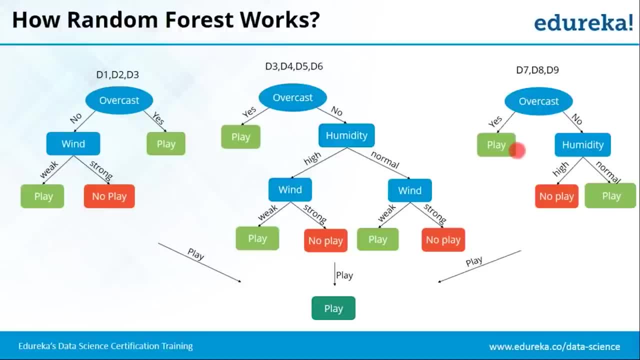 So three different subsets, three different decision trees, three different outcomes and one final outcome after compiling all the results from these three different decision trees. Alright, so I hope this gives a better perspective, a bit understanding of random forest, Like how it really works. All right, 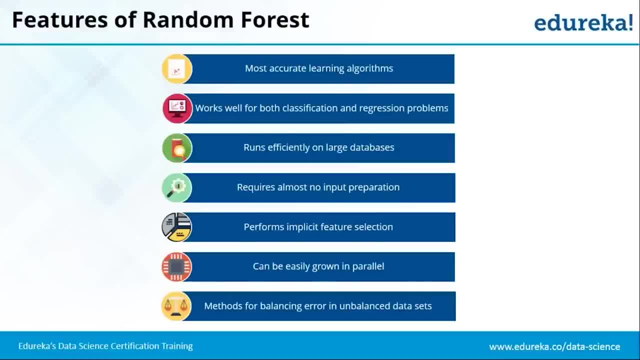 So now let's just have a look at various features of random forest, right? So the first and the foremost feature is that it is one of the most accurate learning algorithms, right? So why it is so? because single decision trees are actually prone to having high variance or high bias. 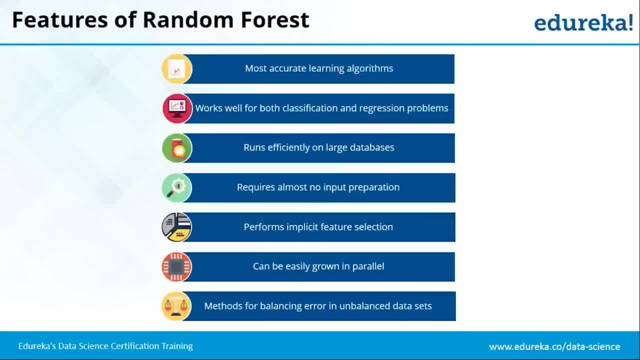 and, on the contrary, actually random forests. it averages the entire variance across The decision trees. So let's say, if the variance is, say, X for decision tree but for random forest, let's say we have implemented n number of decision trees. Parallely: 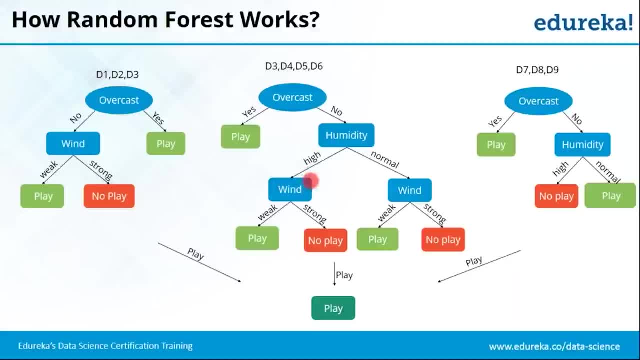 else. Okay, I am making improvement. Humidity was high, but wind was too strong. then you would not go out and play the match Right now. let us look at the second daughter node of humidity. if the humidity was normal And the wind was weak, then you will definitely go out and play the match. as you won't go out and play the match, 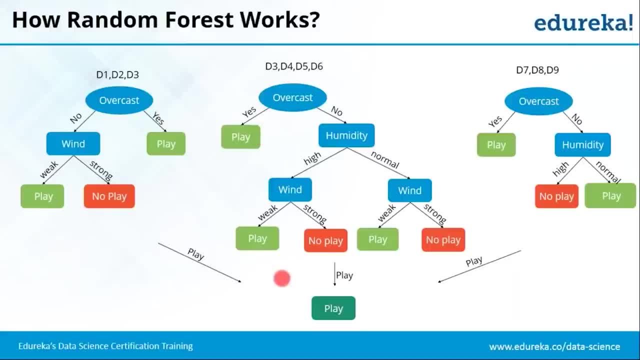 So here, if you look at the final result, Then the ratio of plays to no play is 3 is to 2. then again the final outcome is: actually play right. So from second subset we get the final decision of play. now Let us look at our third subset, which consists of d7 till d9. 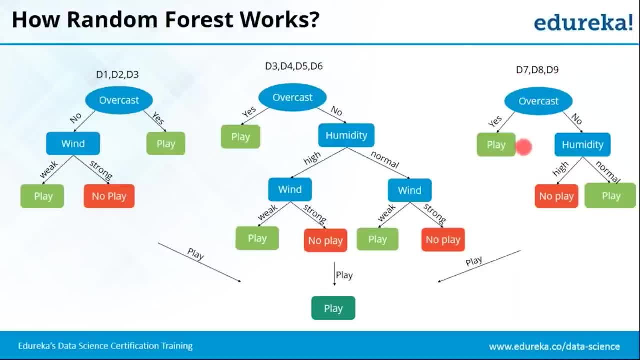 Here. if, again, the overcast is yes, then you will play a match, else You will go and check out for humidity and if the humidity is really high then you won't play the match, else You will play the match again. the probability of playing the matches. 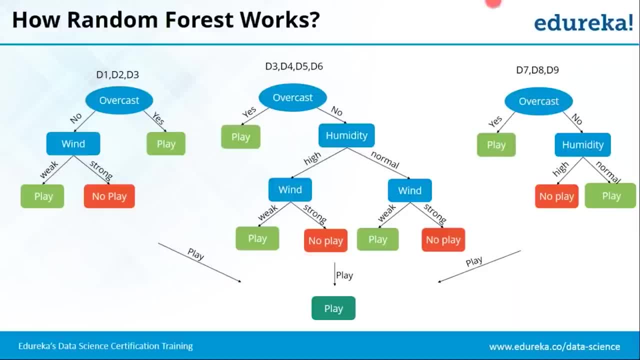 Yes, because the ratio of no play is 2 is to 1. Right, so three different subsets, three different decision trees, three different outcomes and One final outcome after compiling all the results from these three different decision trees. All right, so I hope this gives a better perspective, a bit understanding of random forest, like how it really works. 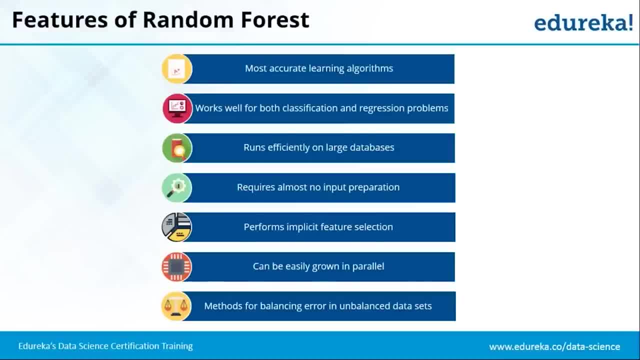 All right. so now let's just have a look at various features of random forest, right? So the first and the foremost feature is that it is one of the most accurate learning algorithms, right? so why it is so? because single decision trees are actually prone to having high variance or high bias, and 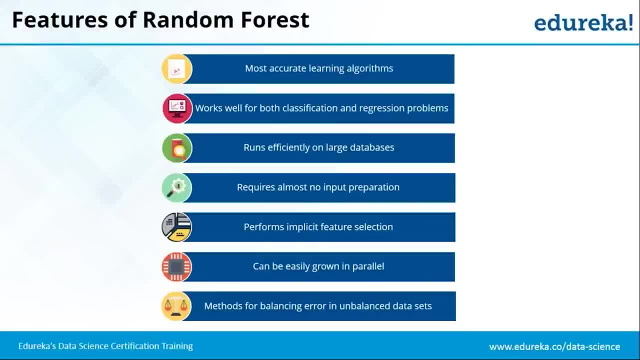 On the contrary, actually random forest, it averages the entire variance across the decision trees. So let's say, if the variance is, say, X for decision tree but for random forest, Let's say we have implemented n number of decision trees, Parallely, so my entire. 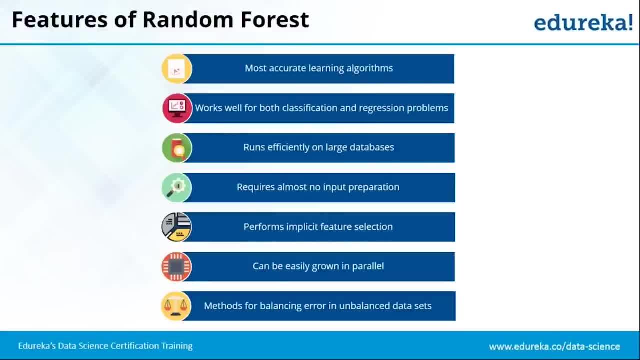 Variance gets averaged upon and my final variance actually becomes X upon n. So that is how the entire variance actually goes down, as compared to other algorithms right now. second most important feature is that it works well for both classification and regression problems and By far I have come across, this is one and the only algorithm which works equally well for both of them. be it. 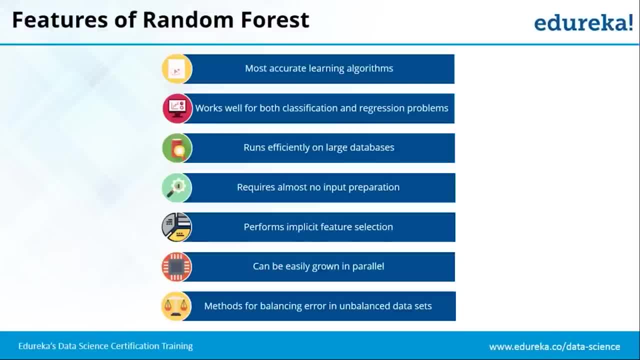 So my entire variance gets averaged upon and my final variance actually becomes X upon n. So that is how the entire variance actually goes down as compared to other algorithms right Now. second most important feature is that it works well for both Classification and regression problems and by far I have come across. 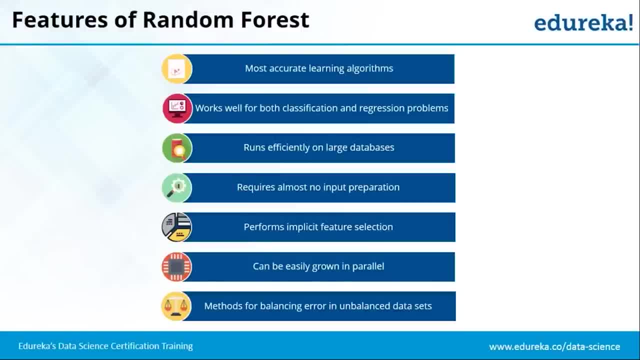 This is one and the only algorithm which works equally well for both of them, Be it classification kind of problem or a regression kind of problem, right, Then it really runs efficient on large databases. So basically it's really scalable, Even if you work for the lesser amount of database or if you work for really huge volume of data. 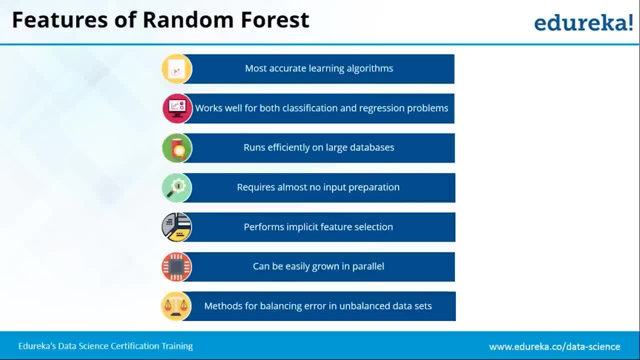 right, So that's A very good part about it. Then, the fourth most important point is that it requires almost no input preparation. Now, why am I saying this? is because it has got certain implicit methods which actually take care and remove all the 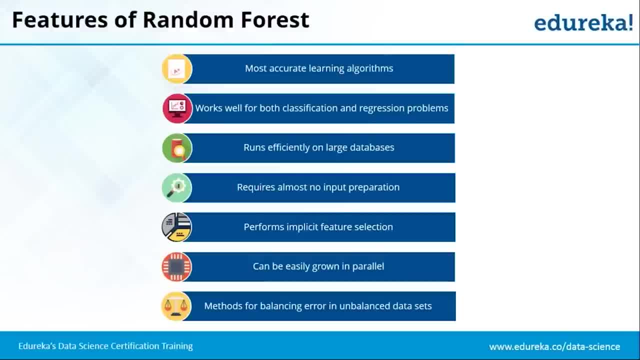 outliers and all the missing data, and you really don't have to take care about all that thing while you are in the stages of input preparation. So random forest is all here to take care of everything else And next is it performs implicit feature selection. 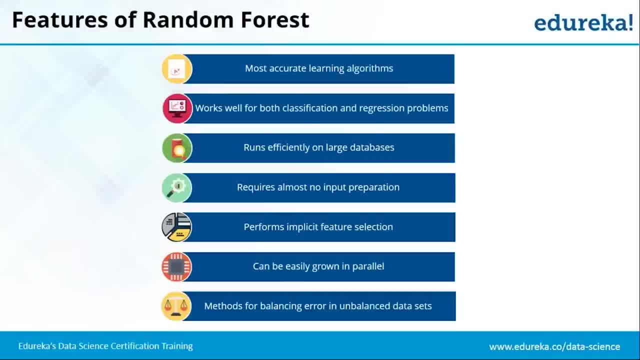 right. So while we are implementing multiple decision trees, so it has got implicit method which will automatically pick up some random features out of all your parameters and then it will go on and implementing different decision trees. So, for example, if you just give one simple command, that all right. 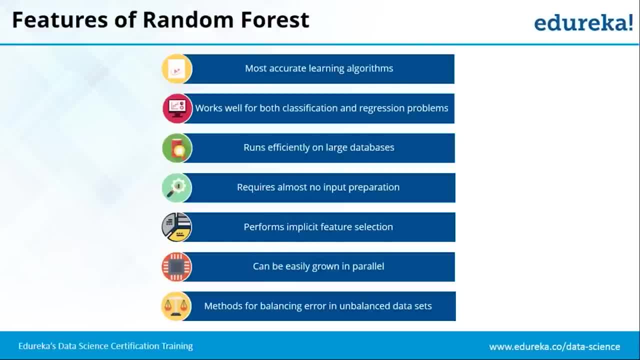 I want to implement 500 decision trees, no matter how, so random forest will Automatically take care and it will implement all those 500 decision trees. and those all 500 decision trees will be different from each other, and this is because it has got implicit methods. 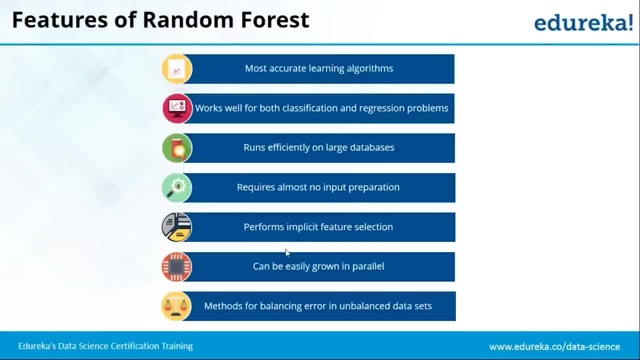 which will automatically collect different parameters itself out of all the variables that you have. right, then it can be easily grown in parallel. why it is so? because we are actually implementing multiple decision trees and all those decision trees are running, or all those decisions trees are actually getting implemented parallelly. 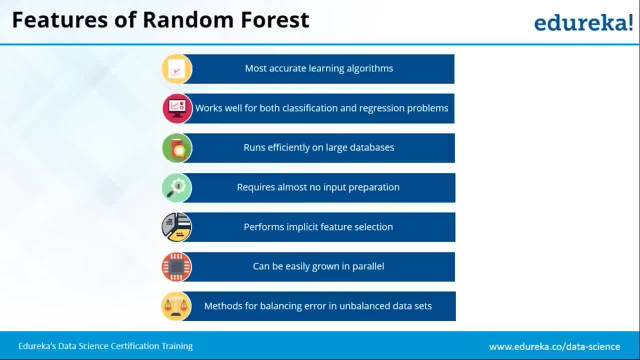 Classification kind of problem or a regression kind of problem, right. Then it really runs efficient on large databases. So basically it's really scalable even if you work for the Lesser amount of database or if you work for really huge volume of data, right. So that's a very good part about it. 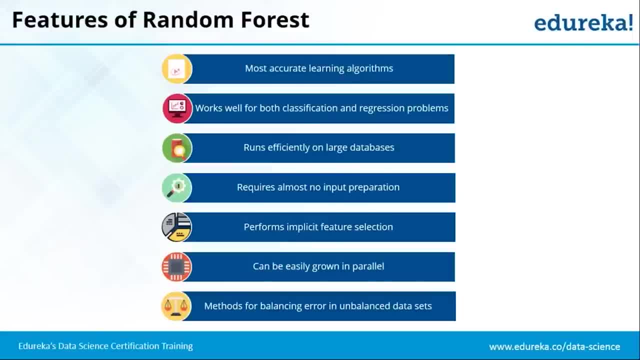 Then the fourth most important point is that it requires almost no input preparation. now, Why am I saying this? is because it has got certain implicit methods which actually take care and remove all the outliers and all the missing data, and You really don't have to take care about all that thing while you are in the stages of input preparation. 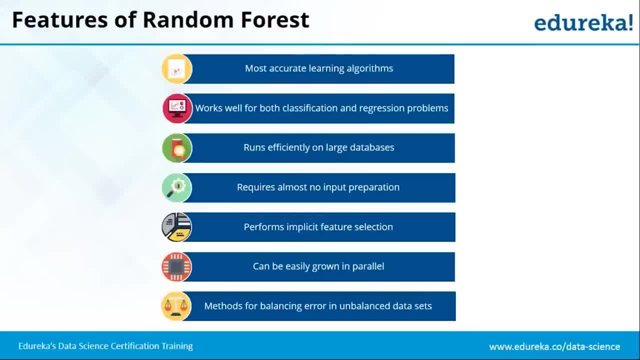 so random forest is all here to take care of everything else, and Next is it performs implicit feature selection, right? So while we are implementing multiple decision trees, so it has got Implicit method which will automatically pick up some random features out of all your parameters And then it will go on and implementing different decision trees. 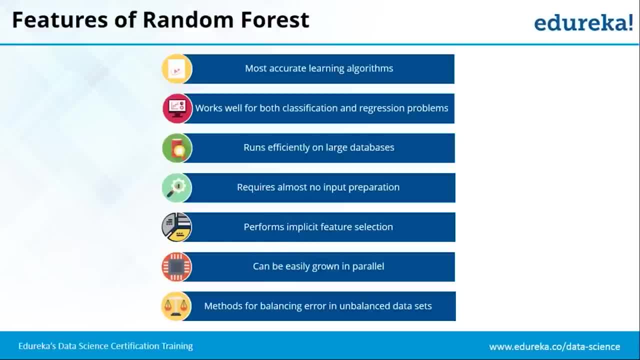 So, for example, if you just give one simple command that all right, I want to implement five hundred decision trees, no matter how, so random forest will automatically take care And it will implement all those five hundred decision trees. and those all five hundred decision trees will be different from each other and 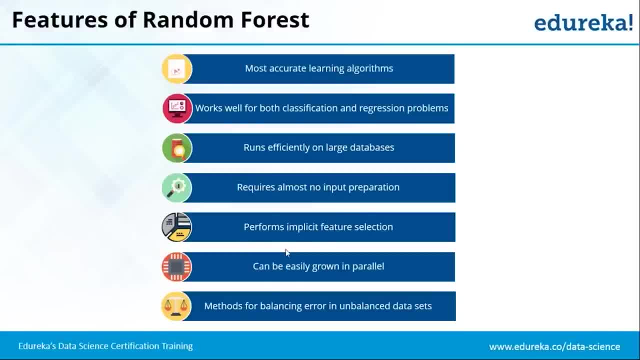 And this is because it has got implicit methods which will automatically collect different parameters Itself out of all the variables that you have. right then it can be easily grown in parallel. Why it is so? because we are actually implementing multiple decision trees and all those Decision trees are running, or all those decisions trees are actually getting implemented parallelly. 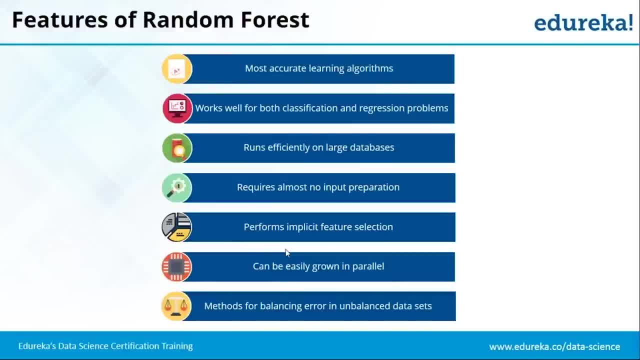 So if you say I want thousand trees to be implemented, So all those thousand trees are getting implemented Pallely. so that is how the competition time reduces down right. and The last point is that it has got methods for balancing error in unbalanced data sets. now. 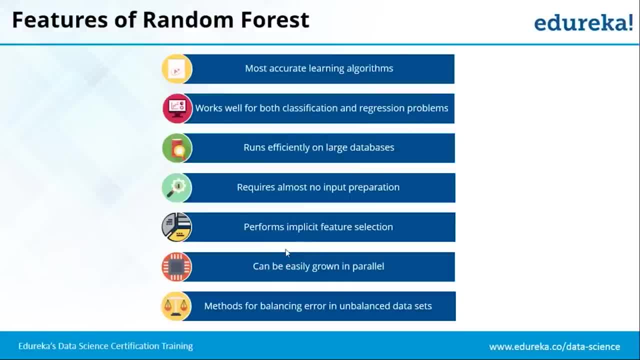 What exactly unbalanced data sets are. let me just give you an example of that. so Let's say you're working on a data set, fine, And you create a random forest model and get 90% accuracy immediately. Fantastic, you think right. so now you start diving deep. you go a little deeper. 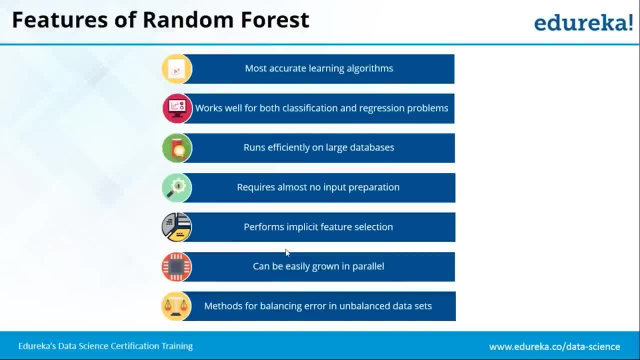 So if you say I want thousand trees to be implemented, so all those thousand trees are getting implemented parallelly. So that is how the competition time reduces down right. And the last point is that it has got methods for balancing error in unbalanced data sets. 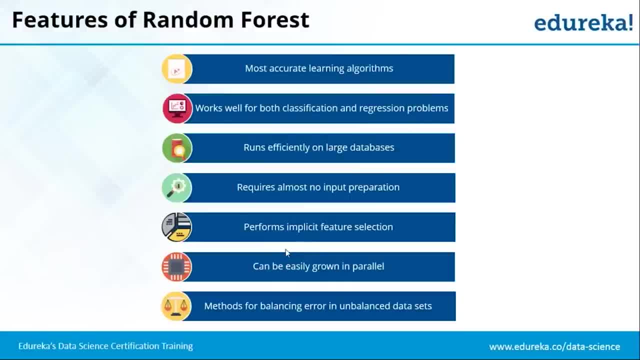 Now what exactly unbalanced data sets are. Let me just give you an example of that. So let's say you're working on a data set right and you create a random forest model and get 90% accuracy immediately. fantastic, You think, right? 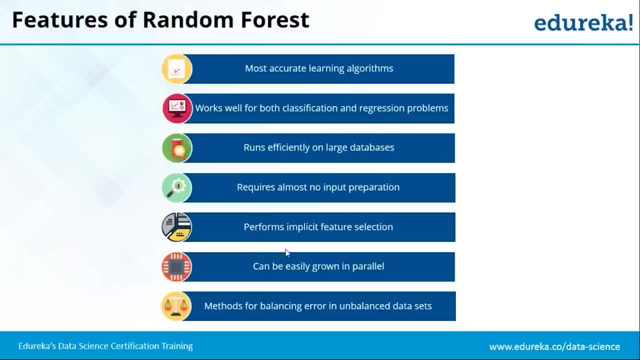 So now you start diving deep, you go a little deeper and you discover that 90% of that data actually belongs to just one class. Damn, your entire data set, your entire decision, is actually biased to just one particular class. So random forest actually takes care of this thing. 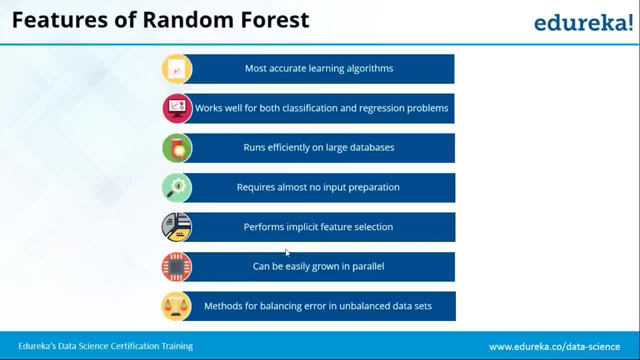 and it is really not biased towards any particular decision tree or any particular variable or any class. So it has got methods which looks after it and they does all the balance of errors in your data sets. So that's pretty much about the features of random forests. 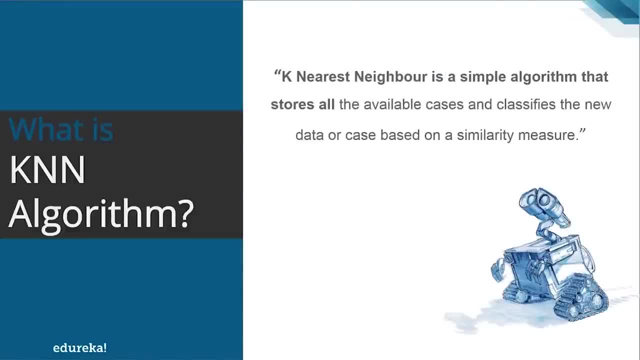 What is Canon Well K nearest neighbor is a simple algorithm that stores all the available cases and classify the new data or case based on a similarity measure. It suggests that if you are similar to your neighbors, then you are one of them, right? 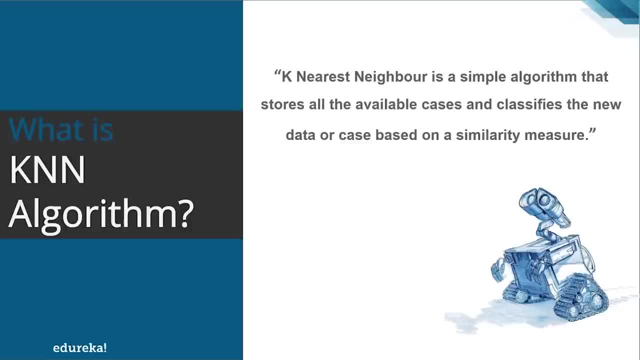 For example, if Apple looks more similar to banana, orange or melon rather than a monkey, rat or a cat, then most likely Apple belong to the group of fruits. All right, Well, in general, Canon is used in search application where you're looking for similar items, that is, when your task is some form of fine items similar to this one. 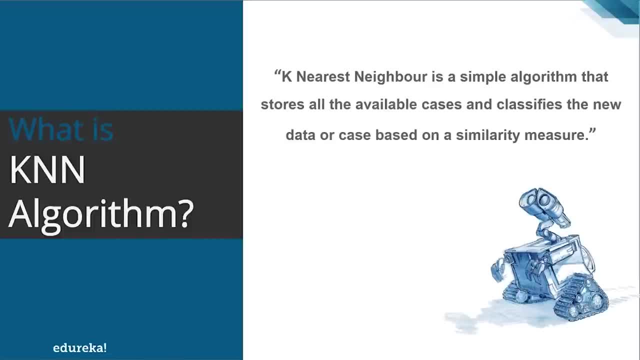 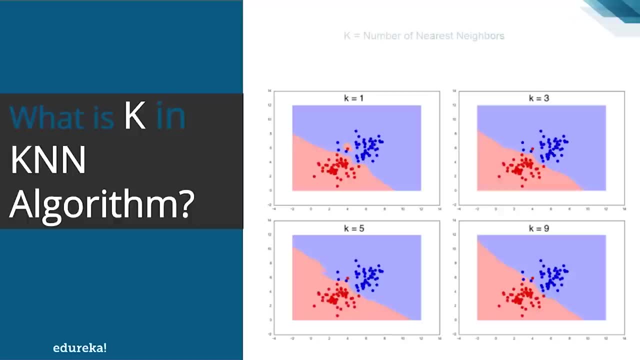 Then you call the search as a Canon search. But what is this K in Canon? Well, this K denotes the number of nearest neighbor which are voting class of the new data or the testing data. For example, if K equal 1, then the testing data are given the same label. as a closest example in the training set, 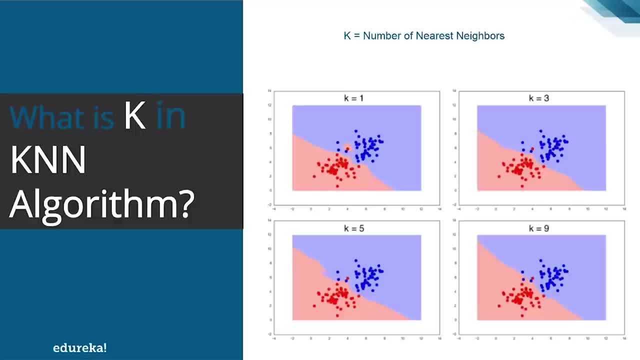 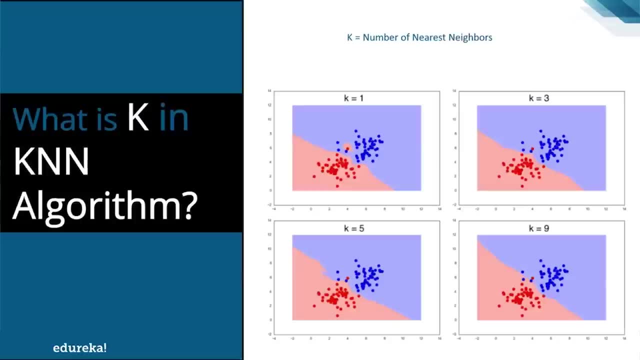 Similarly, if K equal 3, the labels of the three closest classes are checked and the most common label is assigned to the testing data. So this is what a K in Canon algorithm means. So, moving on ahead, Let's see some of the example of scenarios where Canon is used in the industry. 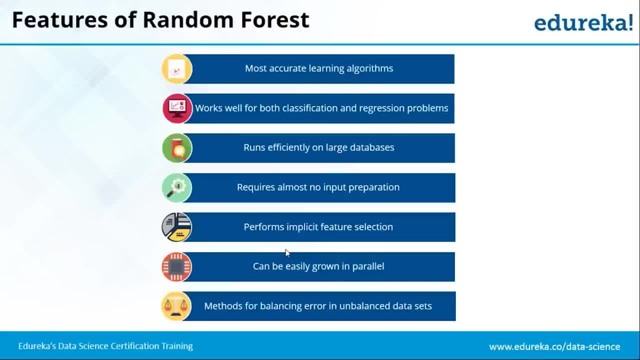 And you discovered that 90% of that data actually belongs to just one class. Damn, your entire data set, your entire decision, is actually biased to just one particular class. So random forest actually takes care of this thing and it is really not biased towards any particular decision tree or 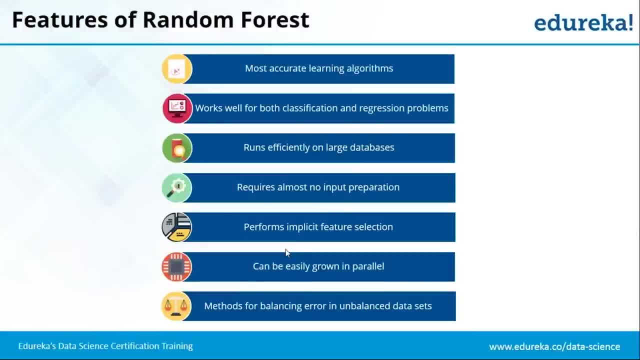 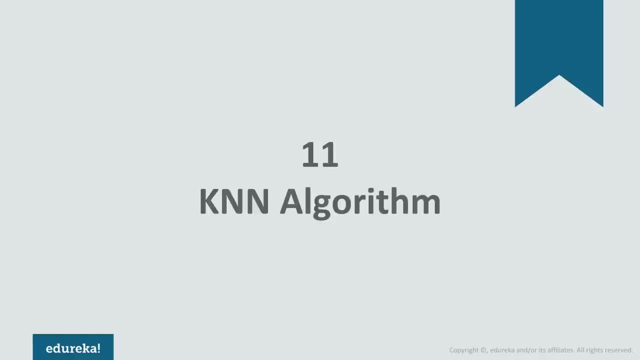 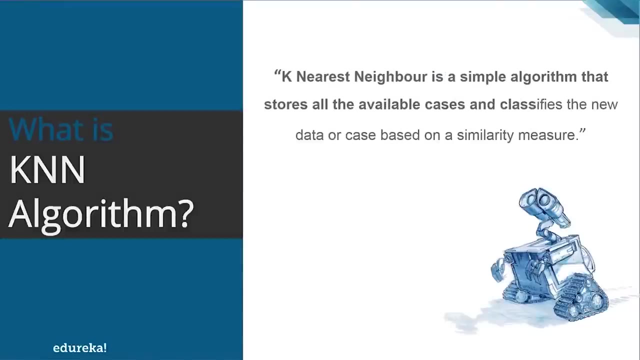 Any particular variable or any class, so it has got methods which looks after it and they does all the balance of errors in your data sets. so that's pretty much about the features of random forests. What is K and N algorithm? Well, K nearest neighbor is a simple algorithm that stores all the available cases and classify the new data or case based on a similarity measure. 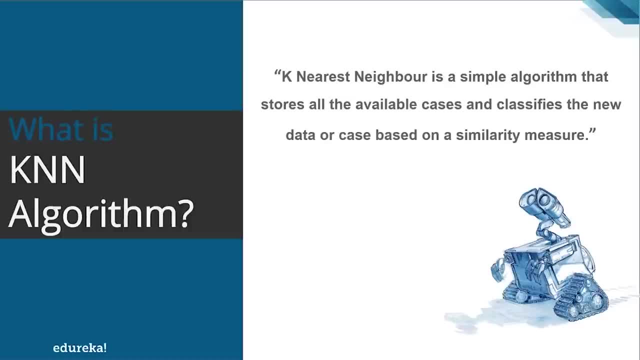 It suggests that if you are similar to your neighbors, then you are one of them, right? For example, if Apple looks more similar to banana, orange or melon rather than a monkey, rat or a cat, then most likely Apple belong to the group of fruits. 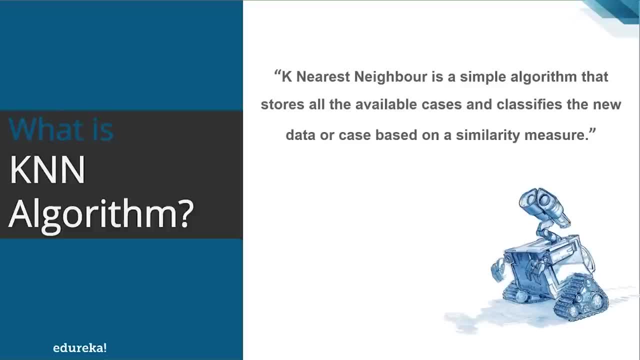 All right. Well, in general, KNN is used in search application where you're looking for similar items, That is, when your task is some form of fine item similar to this one, then you call the search as a KNN search. 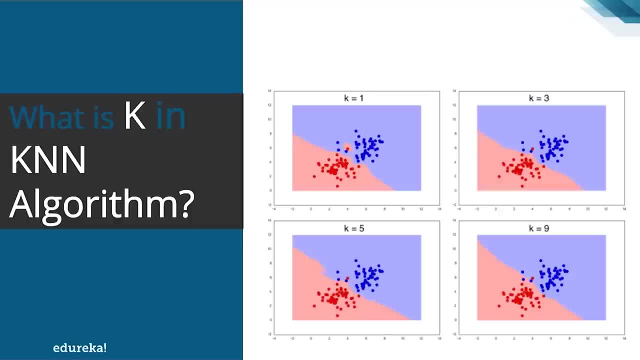 But what is this K in KNN? Well, this K denotes the number of nearest neighbor which are voting class of the new data or the testing data. For example, if K equal one, then the testing data are given the same label as the closest example in the training set. 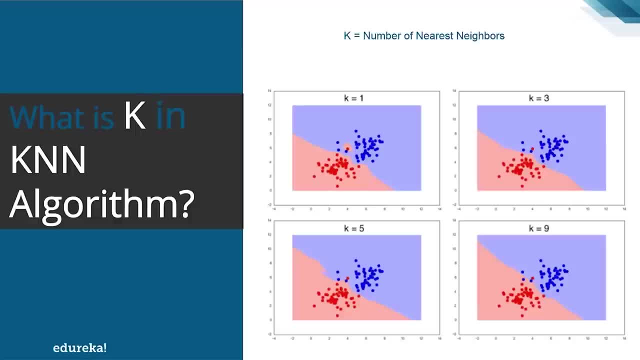 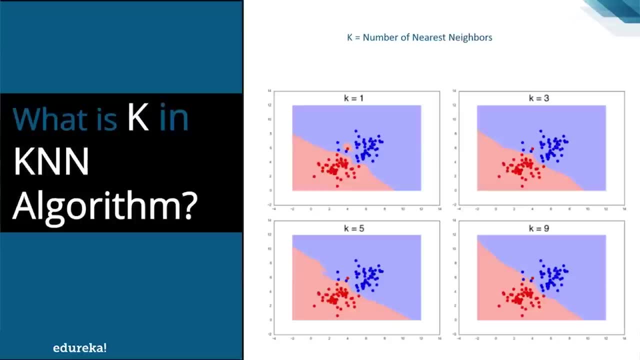 Similarly, if K equal three, the labels of the three closest classes are checked and the most common label is assigned to the testing data. So this is what a KNN algorithm means. So, moving on ahead, let's see some of the example of scenarios. 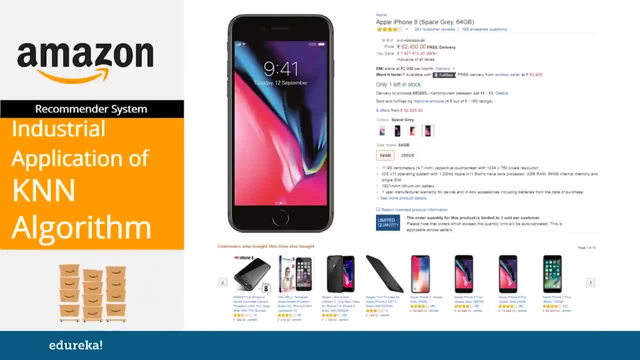 where KNN is used in the industry. So let's see the industrial application of KNN algorithm, starting with recommender system. Well, the biggest use case of KNN search is a recommender system. This recommender system is like an automated form. 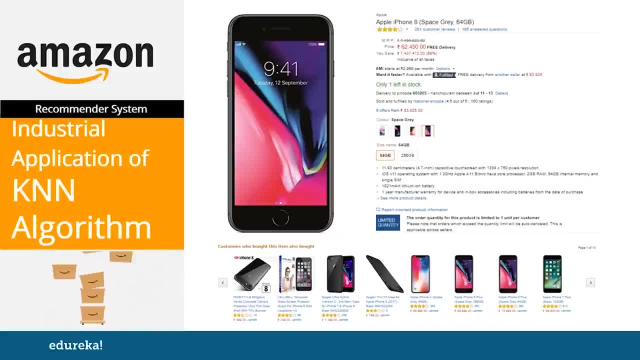 of a shop counter guy When you ask him for a product. not only shows you the product, but also suggest you or displays your relevant set of products which are related to the item you're already interested in buying. This KNN algorithm applies to recommending products. 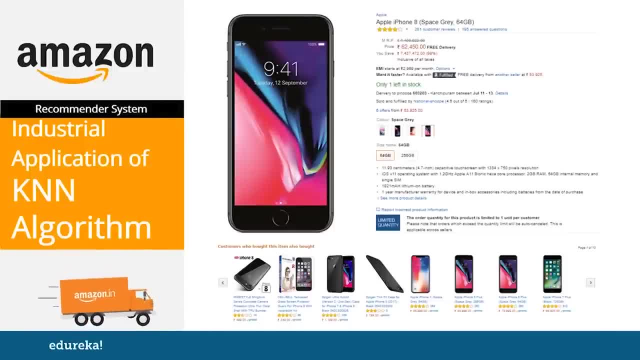 So let's see the industrial application of Canon algorithm, starting with recommender system. Well, the biggest use case of Canon search is a recommender system. This recommender system is like an automated form of a shop counter guy. when you ask him for a product, not only shows you the product but also suggest you or displays your relevant set of products which are related to the item. 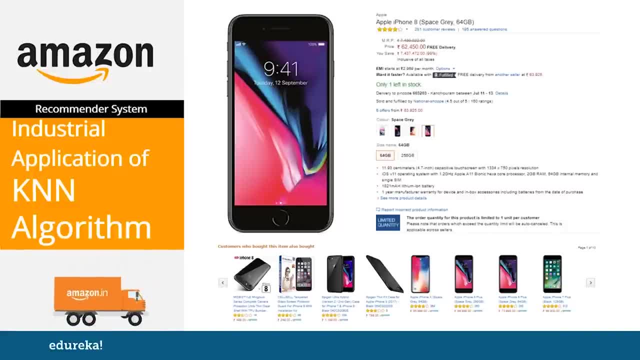 You're already interested in buying. this K in an algorithm applies to recommending products like an Amazon, or for recommending media, Like in case of Netflix, or even for recommending advertisement to display to a user. if I am not wrong, almost all of you must have used Amazon for shopping, right. 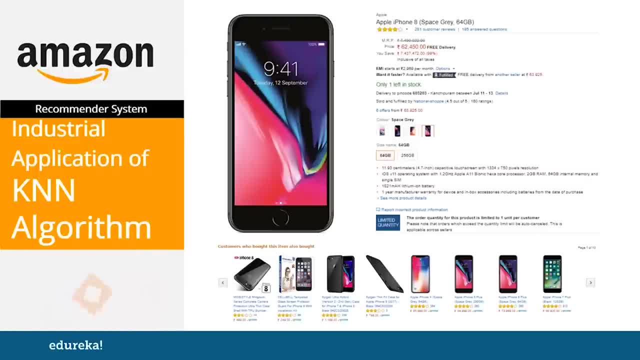 So, just to tell you, more than 35% of amazoncom revenue is generated by its recommendation engine. So what's their strategy? Amazon users recommendation as a targeted marketing tool in both the email campaigns are on most of its website pages. Amazon will recommend many products from different categories based on what your browser, and it will pull those products in front of you. 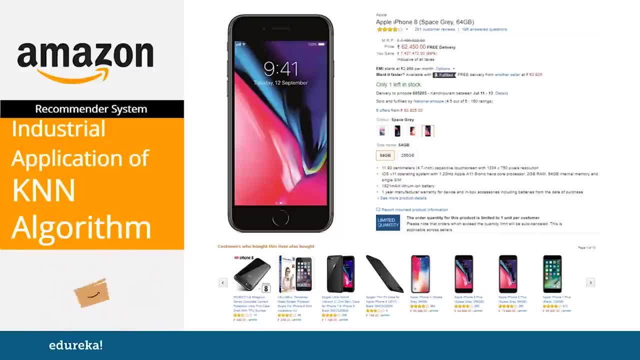 So which are likely to buy, like the frequently bought together option that comes at the bottom of the product page to tempt you into buying the combo. Well, this recommendation has just one main goal, that is, increase average order value or to upsell and cross-sell customers by providing product suggestion based on items in the shopping cart or based on the product. 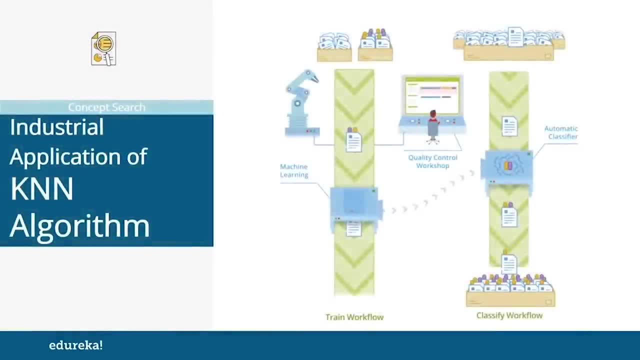 They are currently looking at on-site. So next industrial application of Canon algorithm is concept search, or searching semantically similar documents and classifying documents containing similar topics. So, as you know, the data on the internet is increasing exponentially, every single second. There are billions and billions of documents on the internet. each document on the internet contains multiple concepts that could be a potential concept. 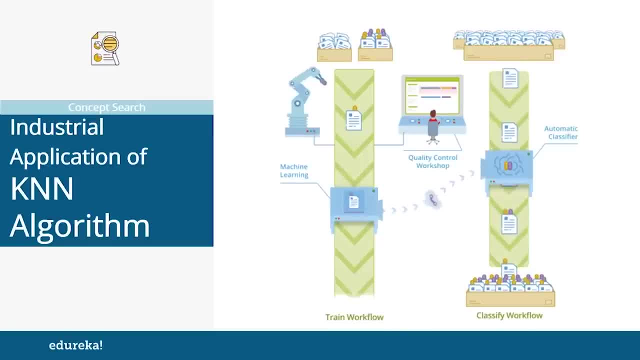 Now there's a situation where the main problem is to extract concept from a set of documents, as each page could have thousands of combination That could be potential concepts. an average document could have millions of concept. combine that to the vast amount of data on the web. 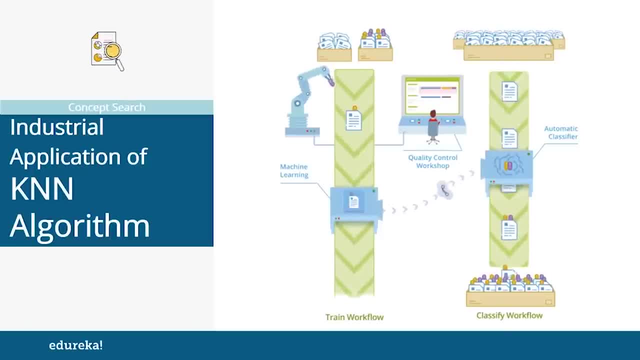 Well, we are talking about an enormous amount of data set And sample. So what we need- a we need to find a concept from the enormous amount of data set and samples, right. So for this purpose we'll be using Canon algorithm. more advanced example could include handwriting detection like an OCR or image of organization, or even video recognition. 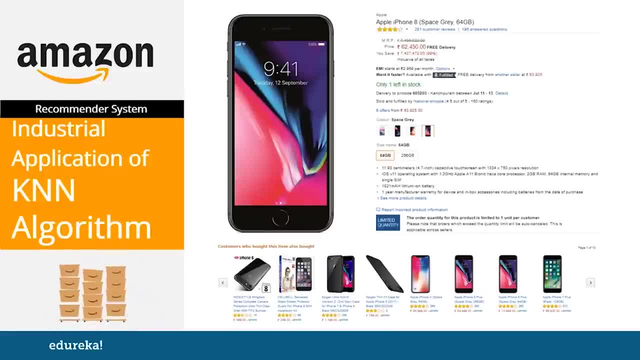 like an Amazon, or for recommending media, like in case of Netflix, or even for recommending advertisement to display to a user. If I'm not wrong, almost all of you must have used Amazon for shopping, right? So just to tell you, more than 35% of amazoncom's revenue. 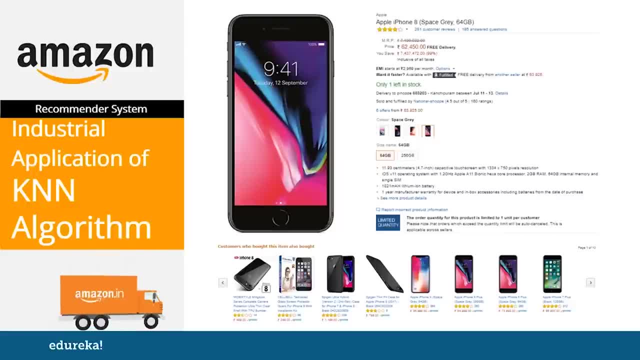 is generated by its recommendation engine. So what's their strategy? Amazon uses recommendation as a targeted marketing tool in both the email campaigns and on most of its website pages. Amazon will recommend many products from different categories based on what your browser, and it will pull those products in front of you. 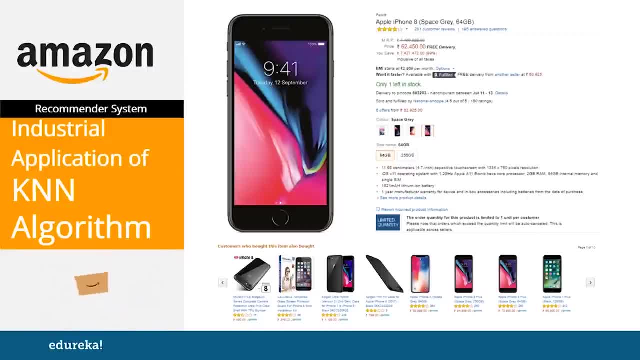 which you're likely to buy, like the frequently bought together option that comes at the bottom of the product page to tempt you into buying the combo. Well, this recommendation has just one main goal, that is, increase average order value or to upsell and cross-sell customers. 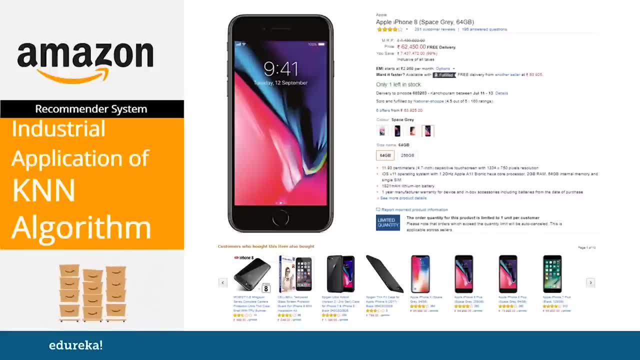 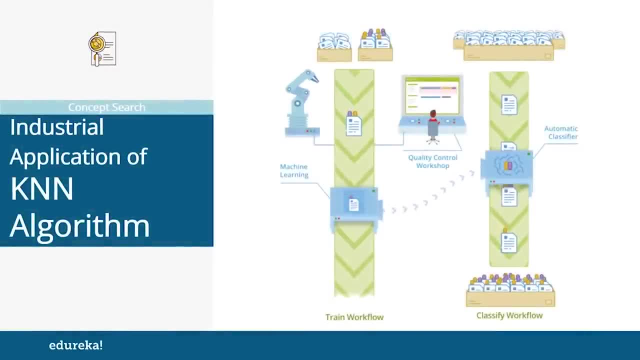 by providing product suggestion based on items in the shopping cart or based on the product they are currently looking at onsite. So next industrial application of KNN algorithm is concept search or searching semantically similar documents and classifying documents containing similar topics. So as you know, 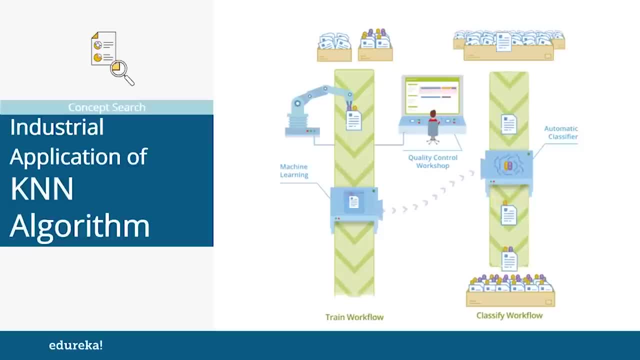 the data on the internet is increasing exponentially every single second. There are billions and billions of documents on the internet. Each document on the internet contains multiple concepts that could be a potential concept. Now there's a situation where the main problem is to extract concept from a set of documents. 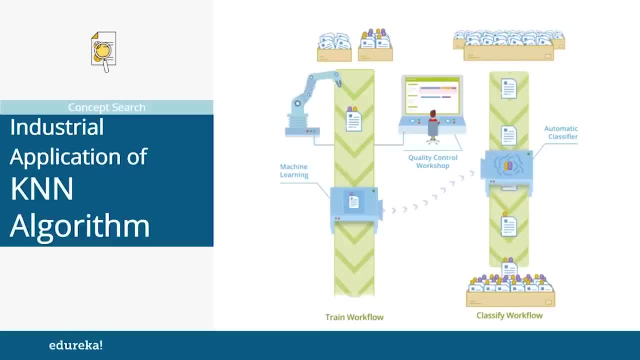 as each page could have thousands of combination. that could be potential concepts. An average document could have millions of concept. combine that to the vast amount of data on the web. Well, we are talking about an enormous amount of data set and sample. So what we need here 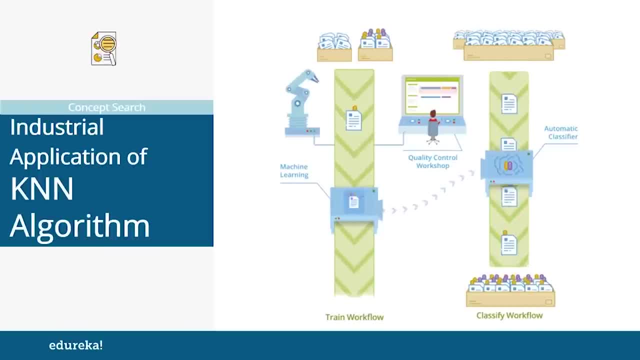 we need to find a concept from the enormous amount of data set and samples right. So for this purpose we'll be using KNN algorithm. More advanced example could include handwriting detection like an OCR or image of organization or even video organization. All right. 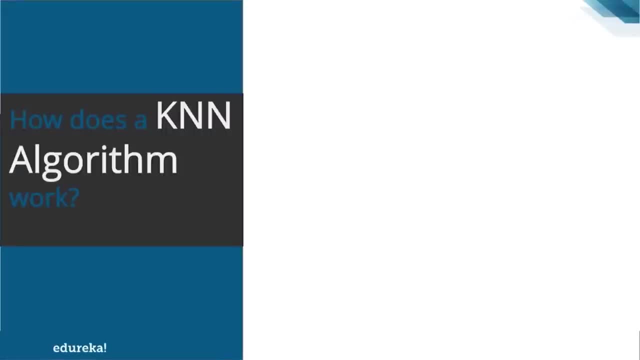 So, now that you know various use cases of KNN algorithm, let's proceed and see how does it work. So how does a KNN algorithm work? Let's start by plotting these blue and orange point on our graph. So these blue points: 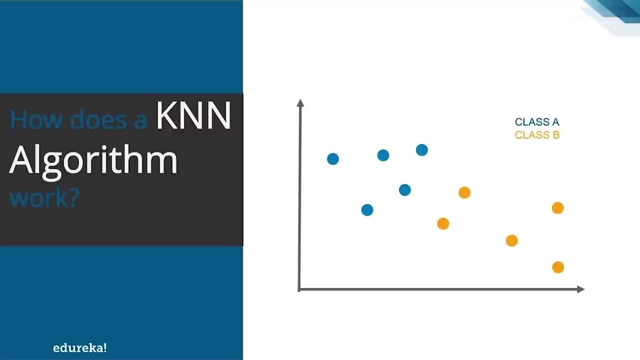 they belong to class A and the orange ones, they belong to class B. Now you get a star as a new point and your task is to predict whether this new point, it belongs to class A or it belongs to class B. So to start the prediction: 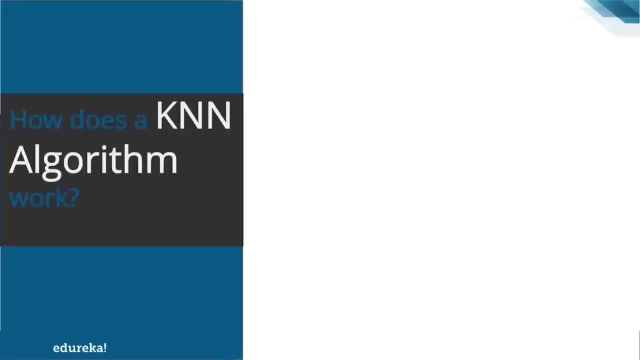 All right. So now that you know various use cases of Canon algorithm, let's proceed and see how does it work. So how does a Canon algorithm work? Let's start by plotting these blue and orange point on our graph. So these blue. 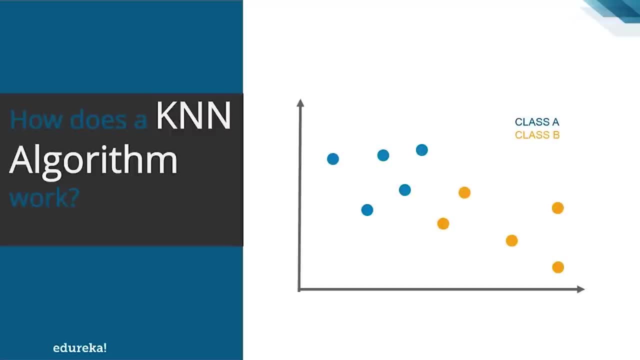 Points: the belong to class a and the orange ones They belong to class B. Now you get a star as a new point and your task is to predict whether this new point, it belongs to class a or it belongs to class B. So to start the prediction: 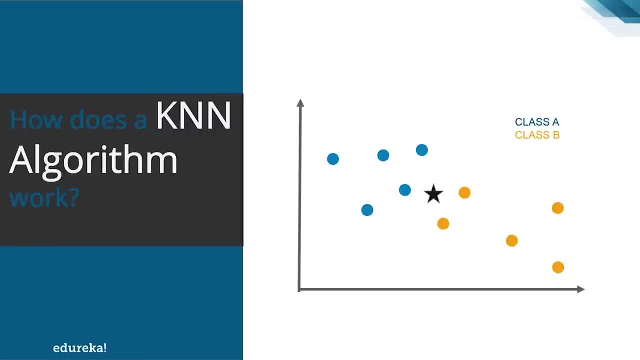 the very first thing that you have to do is select the value of K. Just as I told you, K in Canon algorithm refers to the number of nearest neighbors that you want to select. For example, in this case, K equal 3.. So what does it mean? 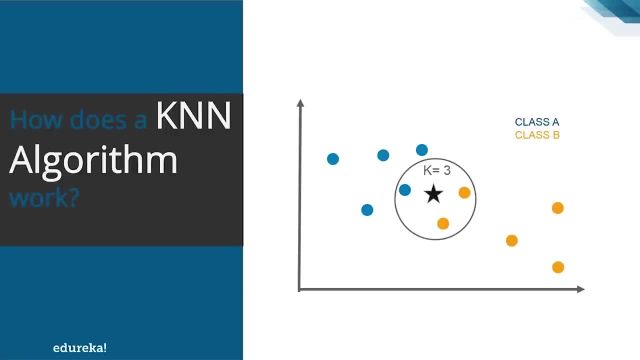 It means that I'm selecting three points which are the least distance to the new point. or you can say I'm selecting three different points which are closest to the star. Well, at this point of time, you can ask: how will you calculate the least distance? 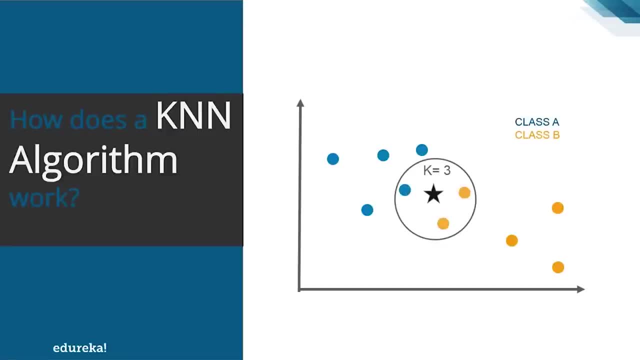 So, once you calculate the distance, you'll get one blue and two orange points, which are closest to the star. Now, since in this case, as we have a majority of orange points, so you can say that for K equal 3, the star belongs to class B. 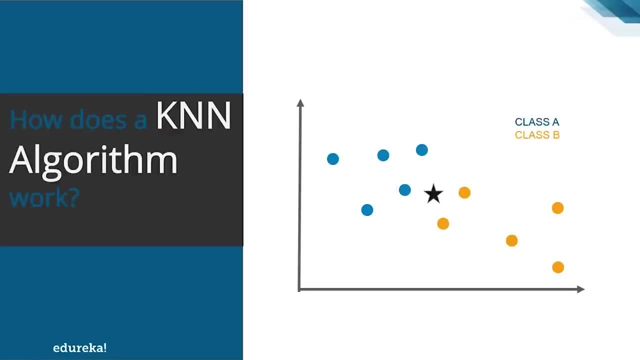 or you can say that the star is more similar to the orange points moving on ahead. Well, what if K equal 6? well, for this case, you have to look for six different points which are closest to the star. So, in this case, after calculating the distance, 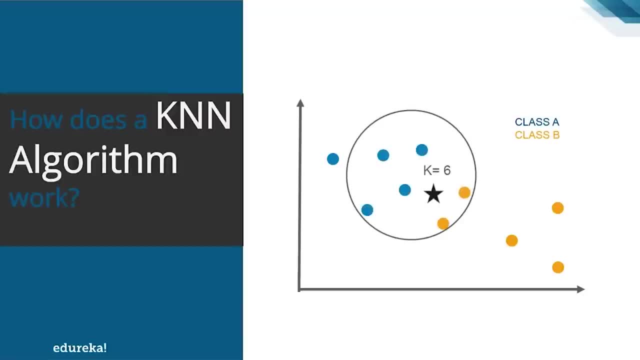 we find that we have four blue points and two orange point, which are closest to the star. Now, as you can see that the blue points are in majority, So you can say that for K equals 6, this star belongs to class A or the star is more similar to blue points. 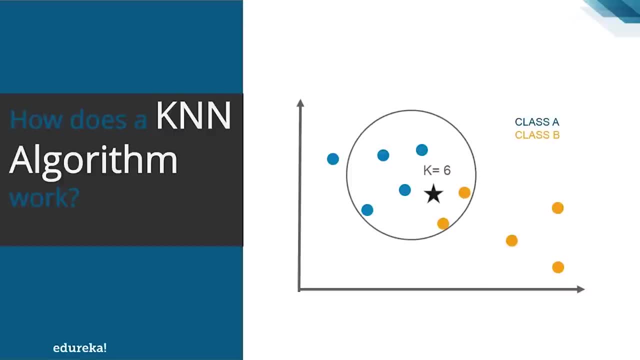 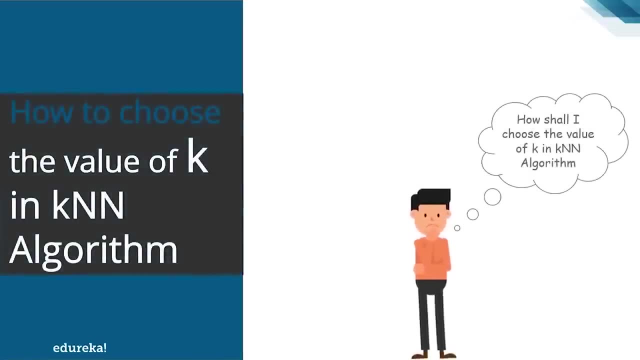 So by now I guess you know how a Canon algorithm work and what is the significance of K in Canon algorithm. So how will you choose the value of K, So keeping in mind this case, the most important parameter in Canon algorithm. So let's see when you build a K nearest neighbor classifier. 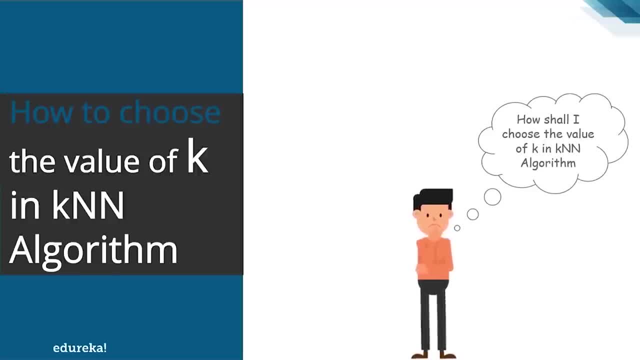 how will you choose a value of K? Well, you might have a specific value of K in mind, or you could divide up your data and use something like cross validation technique to test several values of K in order to determine which works best for your data. 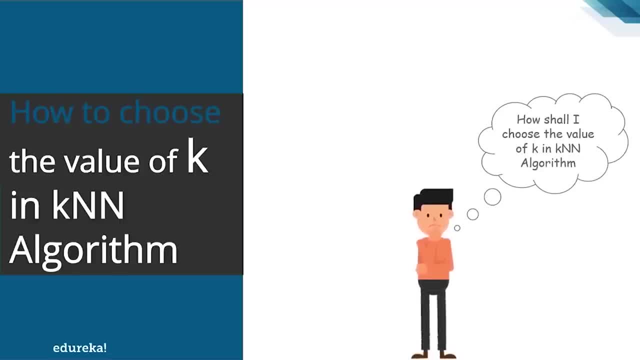 For example, if n equal thousand cases, then in that case the optimal value of K lies somewhere in between 1 to 19,. but is unless you try it, You cannot be sure of it. So you know how the algorithm is working on a higher level. 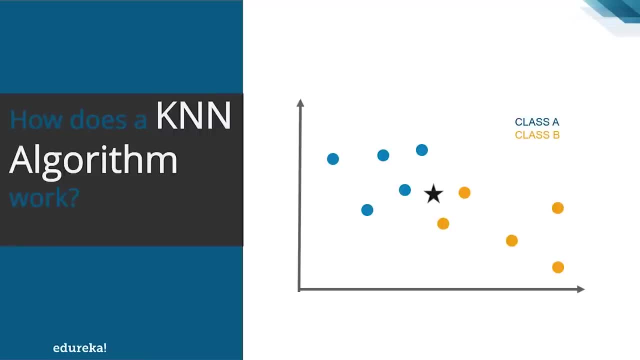 the very first thing that you have to do is select the value of K. Just as I told you, K in KNN algorithm refers to the number of nearest neighbors that you want to select. For example, in this case, K equal three. 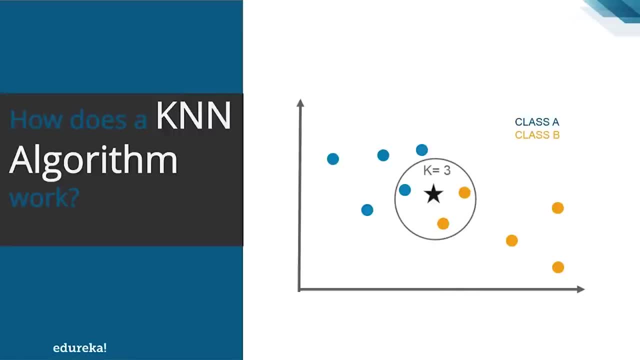 So what does it mean? It means that I'm selecting three points which are the least distance to the new point. or you can say I'm selecting three different points which are closest to the star. Well, at this point of time, you can ask. 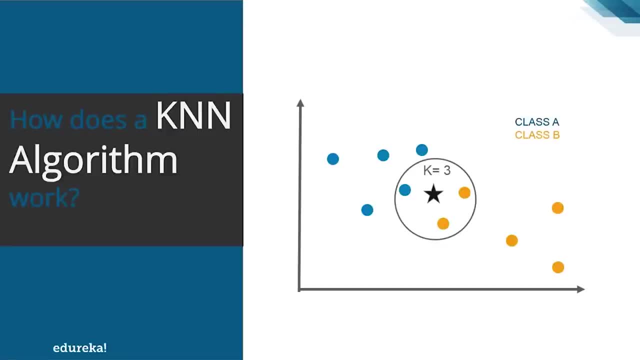 how will you calculate the least distance? So, once you calculate the distance, you'll get one blue and two orange points, which are closest to the star. Now, since in this case, as we have a majority of orange points, so you can say that for K equal three. 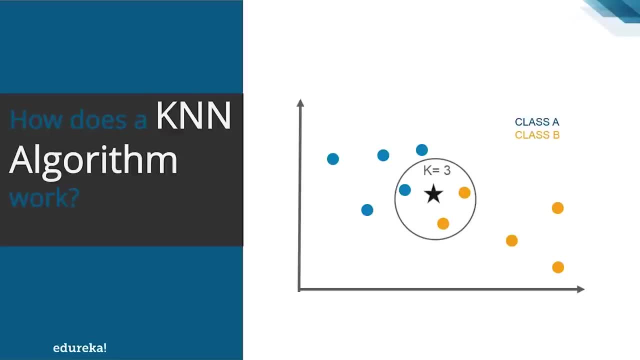 the star belongs to class B, or you can say that the star is more similar to the orange points Moving on ahead. Well, what if K equal to six? Well, for this case, you have to look for six different points which are closest to the star. 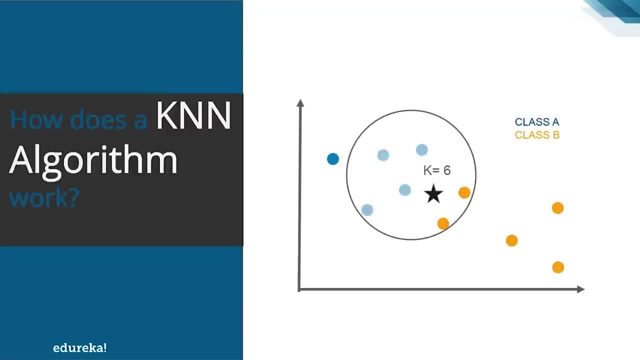 So, in this case, by calculating the distance, we find that we have four blue points and two orange point, which are closest to the star. Now, as you can see that the blue points are in majority, so you can say that for K equals six. 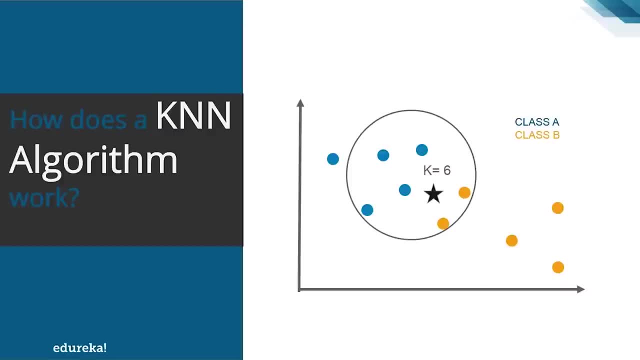 the star belongs to class A, or the star is more similar to blue points. So by now I guess you know how a K-NN algorithm work and what is the significance of K in K-NN algorithm. So how will you choose the value of K? 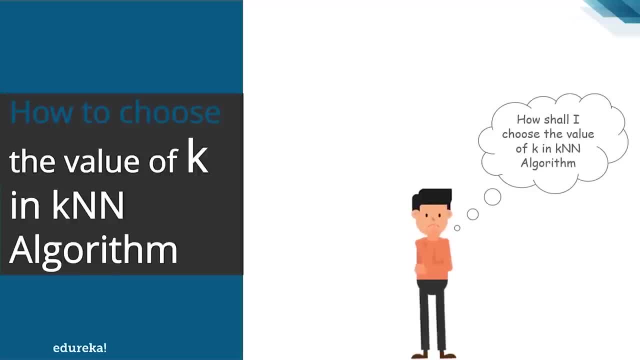 So, keeping in mind this, K is the most important parameter in K-NN algorithm. So let's see: when you build a K nearest neighbor classifier, how will you choose a value of K? Well, you might have a specific value of K in mind. 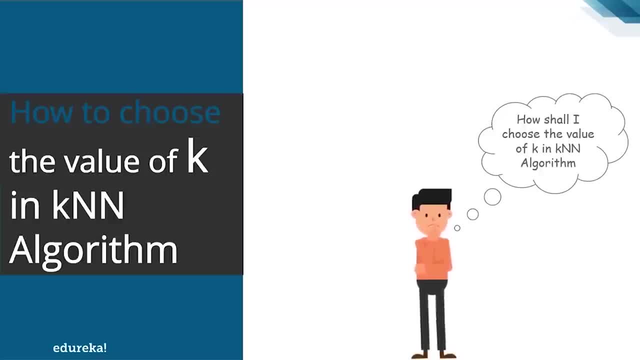 or you could divide up your data and use something like cross validation technique to test several values of K in order to determine which works best for your data. For example, if N equal thousand cases, then in that case the optimal value of K lies somewhere in between one to 19.. 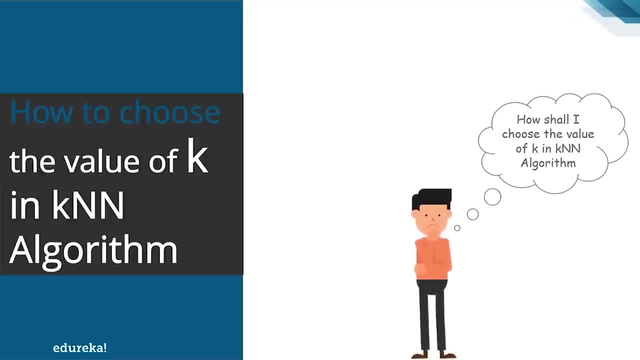 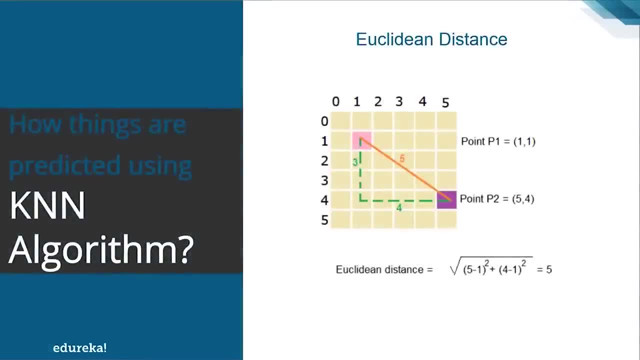 But yes, unless you try it, you cannot be sure of it. So you know how the algorithm is working on a high level. Let's move on and see how things are predicted using K-NN algorithm. Remember I told you, K-NN algorithm uses the least distance measure. 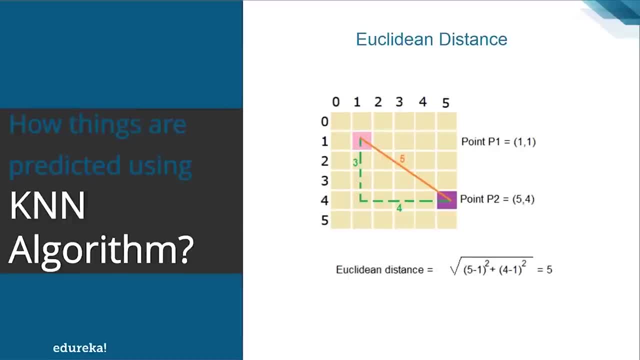 in order to find its nearest neighbors. So let's see how these distances calculated. Well, there are several distance measure which can be used. So, to start with, we'll mainly focus on Euclidean distance and Manhattan distance in this session. So what is this Euclidean distance? 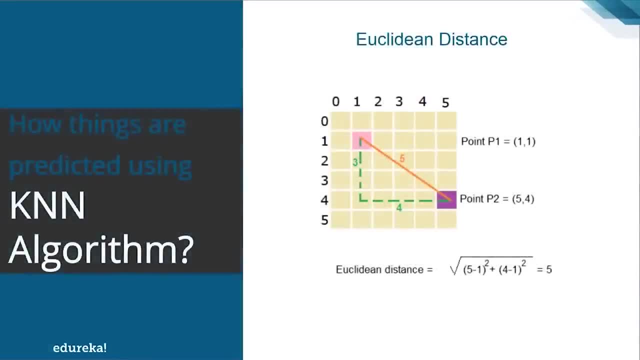 Let's move on and see how things are predicted using Canon algorithm. Remember, I told you, the Canon algorithm uses the least distance measure in order to find its nearest neighbors. So let's see how these distances calculated. Well, there are several distance measure which can be used. 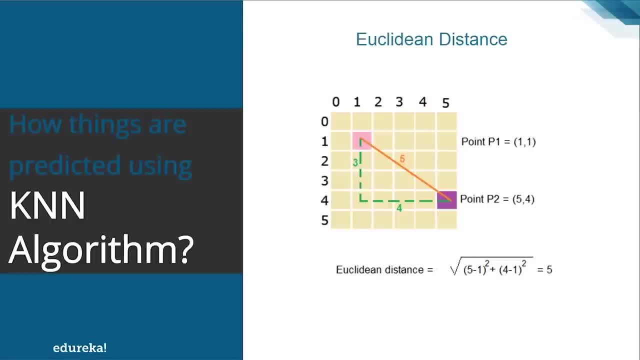 So, to start with, will mainly focus on Euclidean distance and Manhattan distance in this session. So what is this Euclidean distance? Well, this Euclidean distance is defined as the square root of the sum of difference between a new point X And an existing point Y. 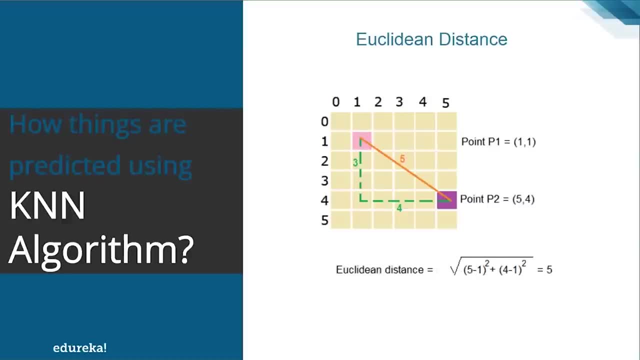 So, for example, here we have point P 1 and P 2. point P 1 is 1: 1 and point P 2 is 5, 4. So what is the Euclidean distance between both of them? So you can say that Euclidean distance is a direct distance. 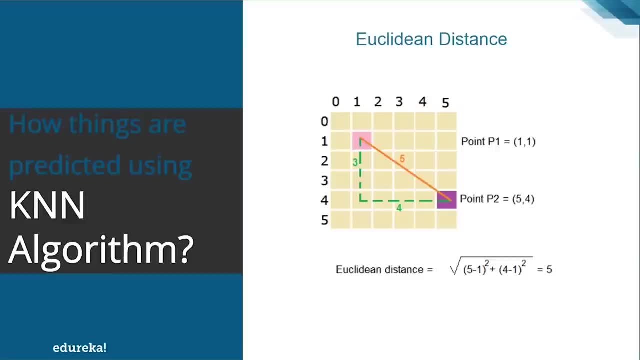 between two points. So what is the distance between the point P 1 and P 2?? So we can calculate it as 5 minus 1 whole square plus 4 minus 1 whole square, and we can root it over, which results to 5.. 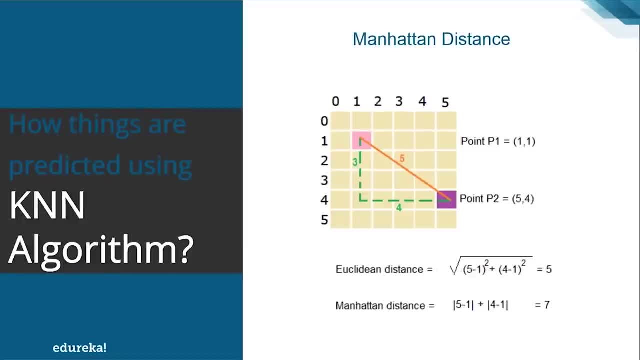 So next is the Manhattan distance. Well, this Manhattan distance is used to calculate the distance between real vector using the sum of their absolute difference. In this case, the Manhattan distance between the point P 1 and P 2 is mod of 5 minus 1 plus mod value of 4 minus 1, which results to 3 plus. 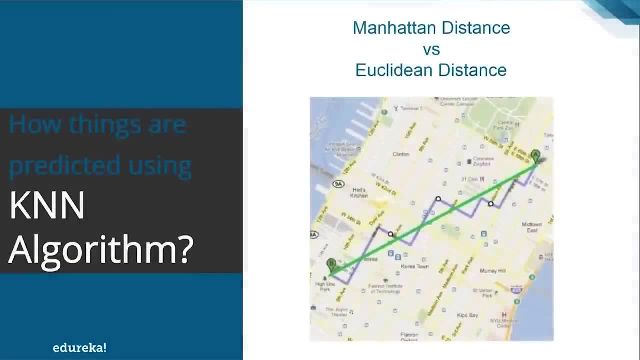 4, that is, 7.. So this slide shows the difference between Euclidean and Manhattan distance from point A to point B. So Euclidean distance is nothing but the direct or the least possible distance between A and B, whereas the Manhattan distance is the distance between A and B measured along the axis at. 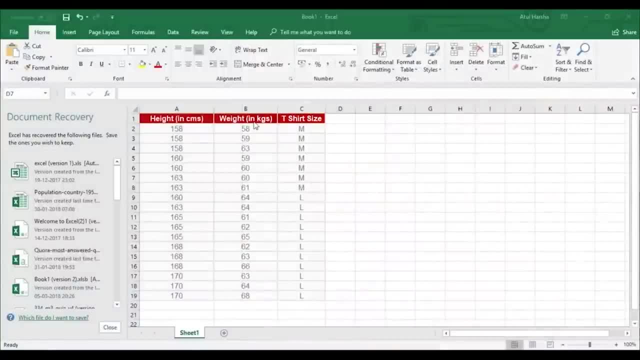 right angle. Let's take an example and see how things are predicted using K-NN algorithm, or how the K-NN algorithm is working. Suppose we have a data set which consists of height, weight and t-shirt size of some customers. Now, when a new customer come, we only have his height and weight. 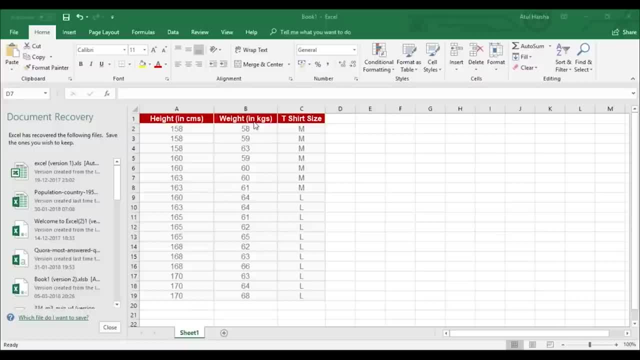 as the information. Now our task is to predict what is the t-shirt size of that particular customer. So for this will be using the K-NN algorithm. So, the very first thing, what we need to do, We need to calculate the Euclidean distance. 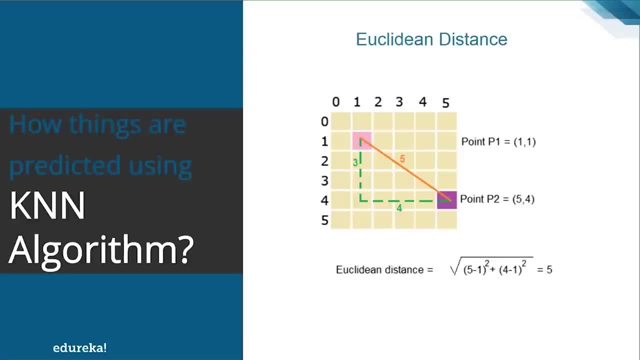 Well, this Euclidean distance is defined as a square root of the sum of difference between a new point X and an existing point Y. So, for example, here we have point P1 and P2.. Point P1 is one one and point P2 is five four. 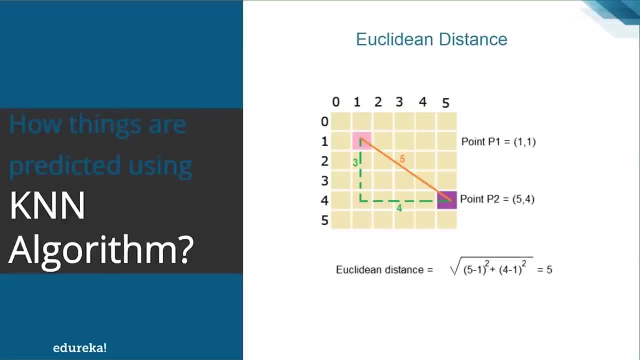 So what is the Euclidean distance between both of them? So you can say that Euclidean distance is a direct distance between two points. So what is the distance between the point P1 and P2?? So we can calculate it as five minus one whole square. 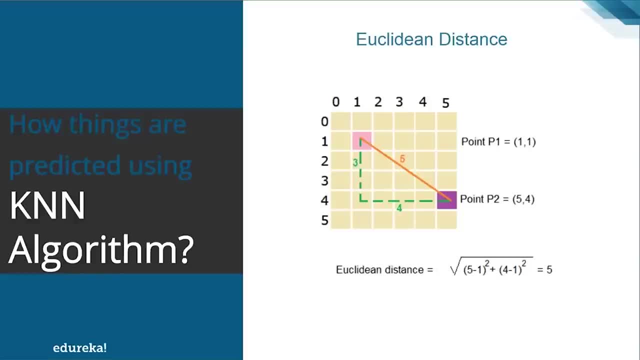 plus four, minus one whole square, and we can root it over, which results to five. So next is the Manhattan distance. Well, this Manhattan distance is used to calculate the distance between real vector using the sum of their absolute difference, In this case the Manhattan distance. 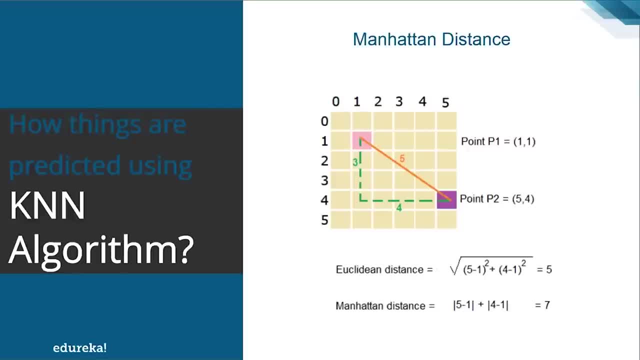 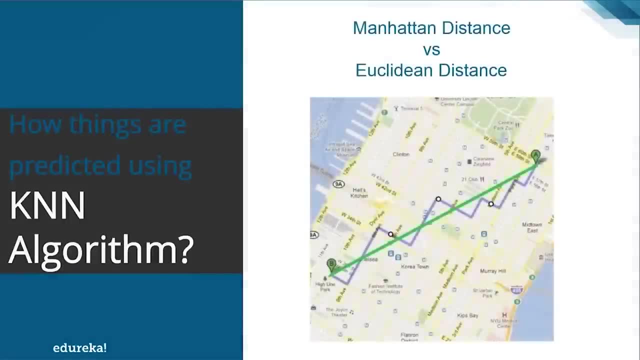 between the point P1 and P2 is mod of five minus one plus mod value of four minus one, which results to three plus four, that is seven. So this slide shows the difference between Euclidean and Manhattan distance from point A to point B. 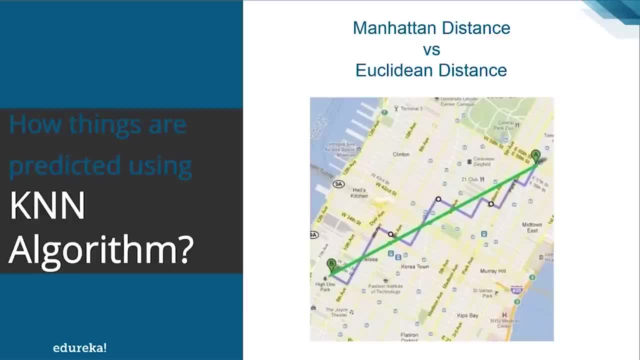 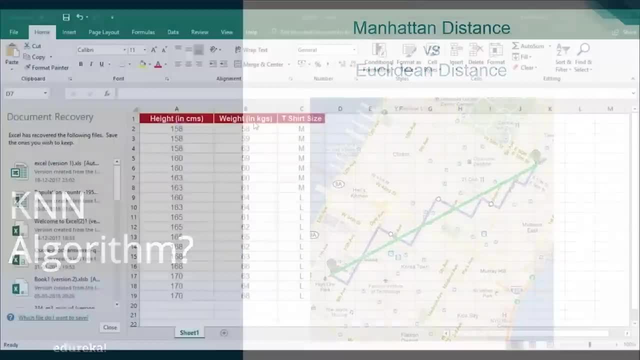 So Euclidean distance is nothing but the direct or the least possible distance between A and B, Whereas the Manhattan distance is a distance between A and B measured along the axis at right angle. Let's take an example and see how things are predicted using K-NN algorithm. 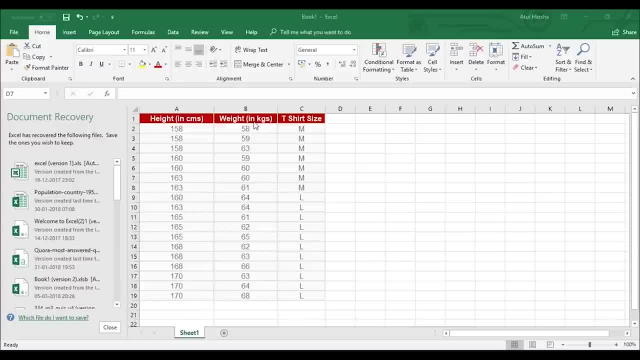 or how the K-NN algorithm is working. Suppose we have a data set which consists of height, weight and t-shirt size of some customers. Now, when a new customer come, we only have his height and weight as the information. Now our task is to predict what is the t-shirt size. 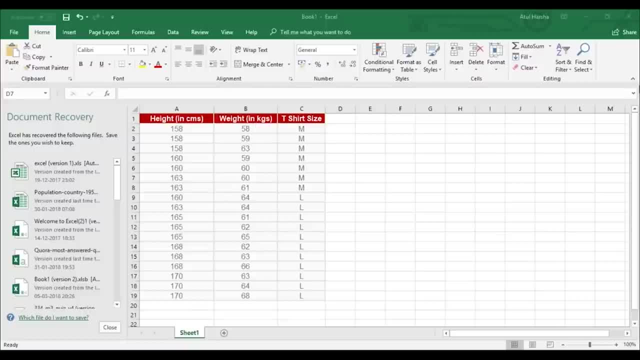 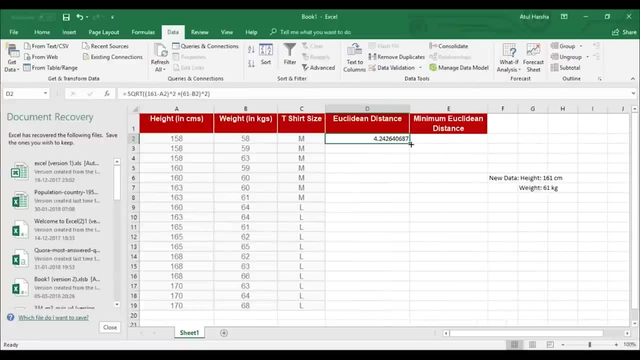 of that particular customer. So for this we'll be using the K-NN algorithm. So the very first thing, what we need to do, we need to calculate the Euclidean distance. So now that you have a new data, of height: 161 centimeter. 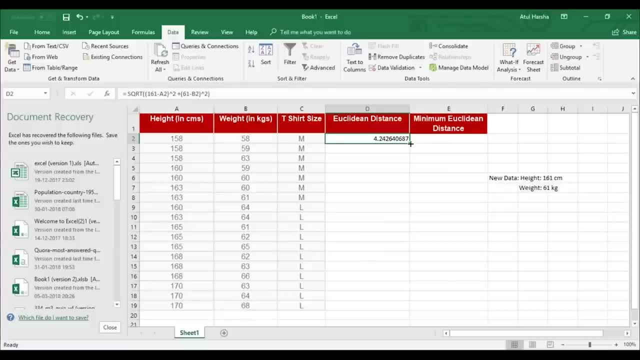 and weight as 61 kg. so the very first thing that we'll do is we'll calculate the Euclidean distance, which is nothing but the square root of 161 minus 158 whole square, plus 61 minus 58 whole square, and square root of that is 4.24.. 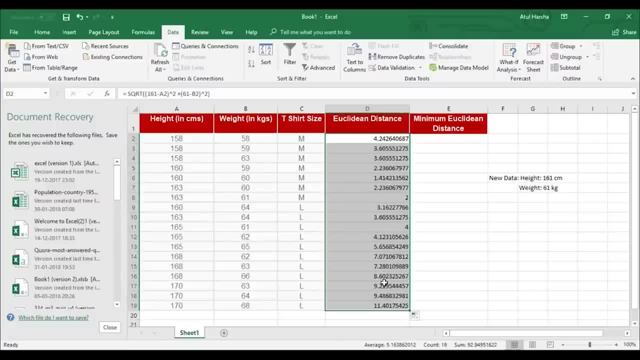 Let's drag and drop it. So these are the various Euclidean distance of other points. Now let's suppose K equal to five. then the algorithm what it does? it searches for the five customer closest to the new customer. that is more similar to the new data. 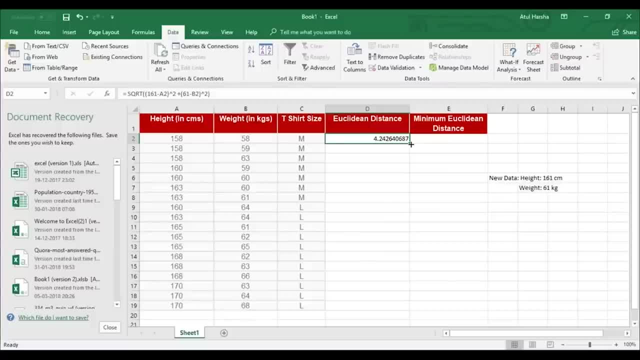 So, now that you have a new data of height- 161 centimeter- and weight as 61 kg, So the very first thing that we'll do is we'll calculate the Euclidean distance, which is nothing but the square root of 161 minus 158 whole square, plus 61 minus 58 whole square, and 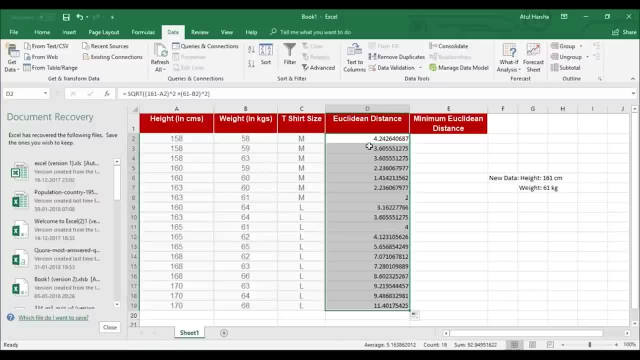 square root of that is 4.24.. Let's drag and drop it. So these are the various Euclidean distance of other points. Now let's suppose K equal to 5. then the algorithm, what it does? it searches for the five customer. 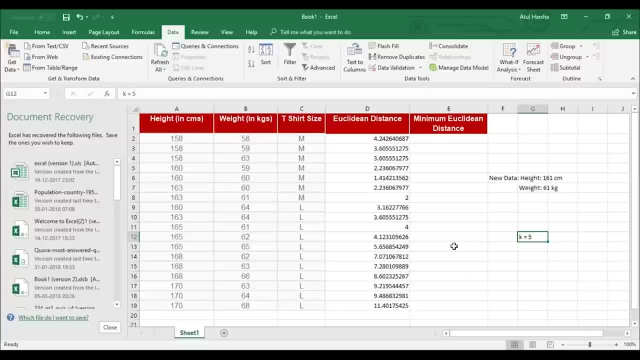 Closest to the new customer. that is more similar to the new data in terms of its attribute for K equal 5.. Let's find the top 5 minimum Euclidean distance. So these are the distance which we are going to use: 1, 2, 3, 4. 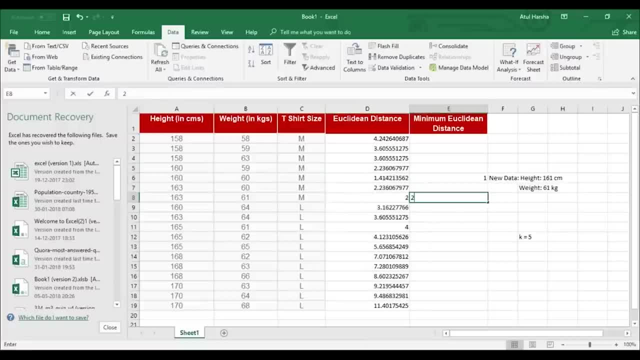 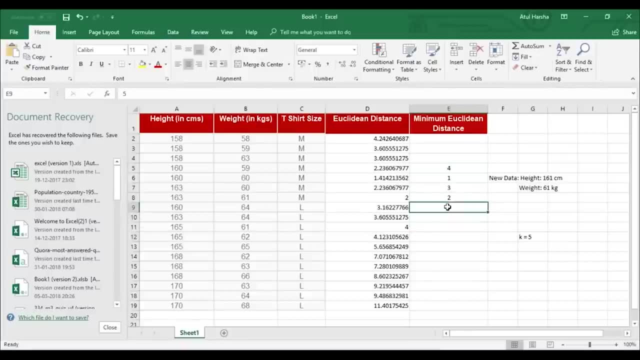 and 5.. So let's rank them in the order: first This is second, is third, then this one is 4 and again this one is 5.. So there's our order. So for K, equal 5, we have four t-shirts which come under size. 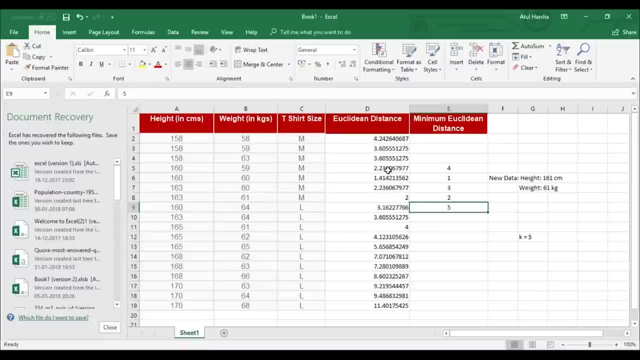 M and one t-shirt which comes under size L. So obviously best guess or the best prediction for the t-shirt- size of height, 161 centimeter and weight, 61 kg- is M, or you can say that our new customer fit into size M. Well, this was all about the theoretical session. 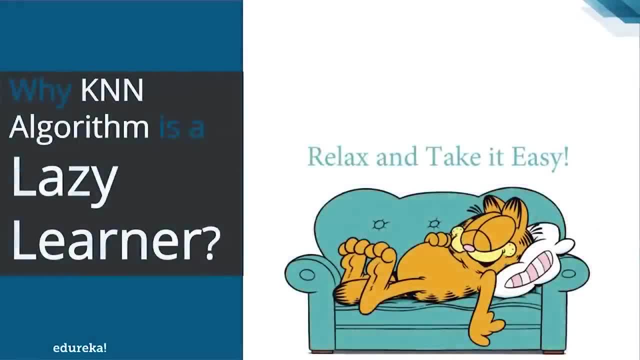 But before we drill down to the coding part, let me just tell you why people call KNN as a lazy learner. Well, KNN, for classification, is a very simple algorithm, but that's not why they are called lazy. KNN is a lazy learner because it doesn't have a discriminative 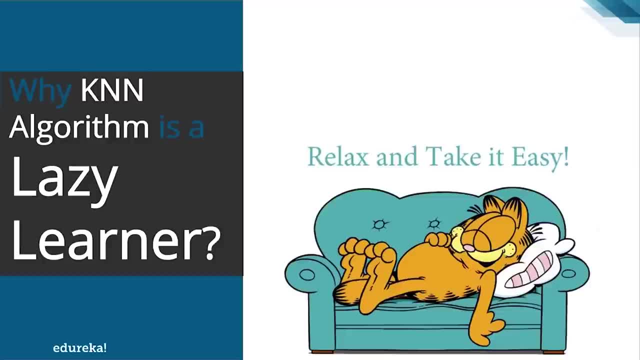 function from the training data, But what it does? it memorizes the training data. There is no learning phase of the model and all of the work happens at the time of prediction is requested. So, as such, there's the reason why KNN is often referred to. 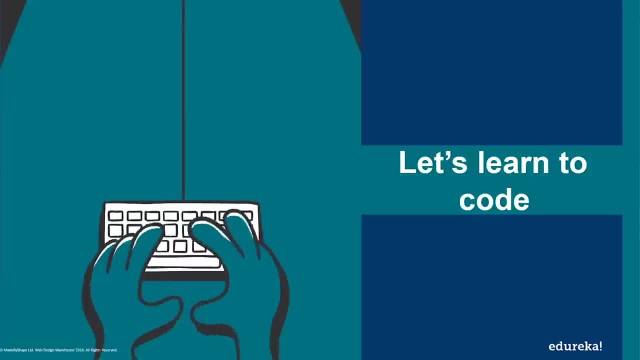 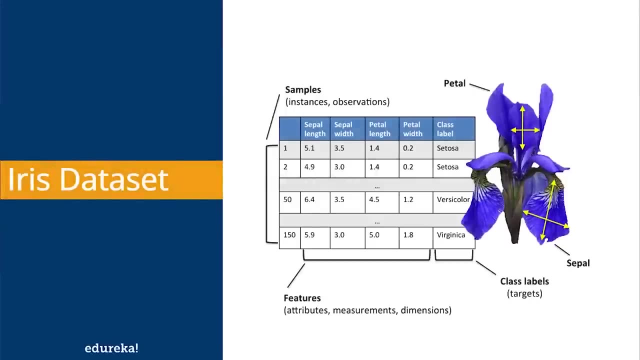 as lazy learning algorithm. So this was all about the theoretical session. Now let's move on to the coding part. So for the practical implementation of the hands-on part, I'll be using the IDIS data set. So this data set consists of 150 observation. 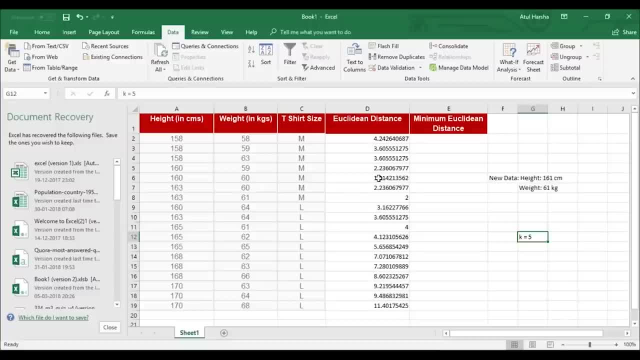 in terms of its attribute For K equal five. let's find the top five minimum Euclidean distance. So these are the distance which we are going to use: one, two, three, four and five. So let's rank them in the order. 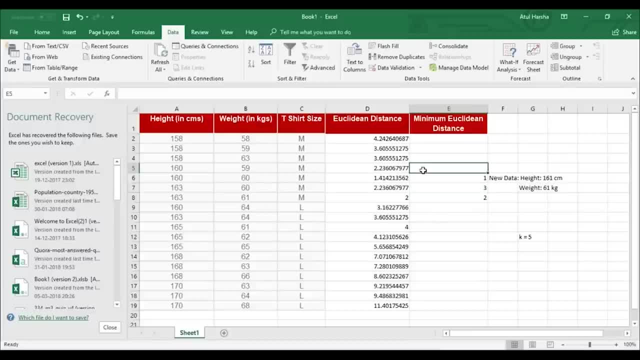 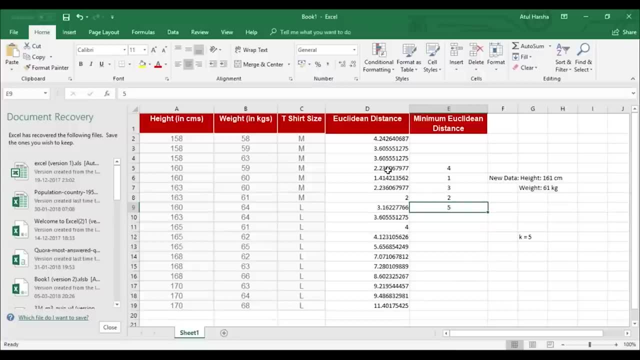 First, this is second, this is third, then this one is four and again this one is five. So there's our order. So for K, equal five. we have four t-shirts which come under size M and one t-shirt which comes under size L. So obviously best guess or the best prediction for the t-shirt size of height 161 centimeter and weight 61 kg- is M, or you can say that our new customer fit into size M. Well, this was all about the theoretical session. 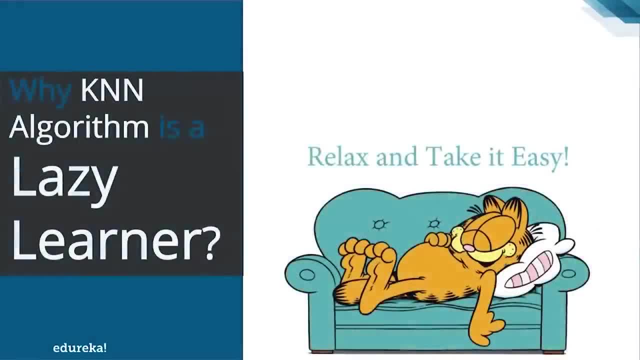 but before we drill down to the coding part, let me just tell you why people call KNN as a lazy learner. Well, KNN for classification is a very simple algorithm, but that's not why they are called lazy. KNN is a lazy learner. 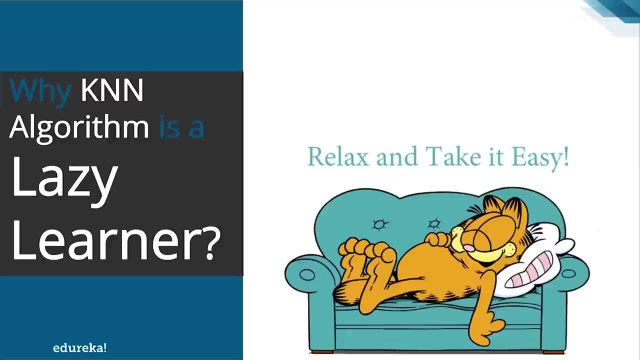 because it doesn't have a discriminative function from the training data, but what it does? it memorizes the training data. There is no learning phase of the model and all of the work happens at the time of prediction is requested, So as such. 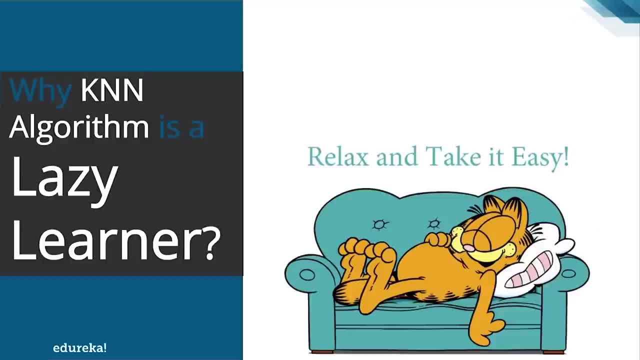 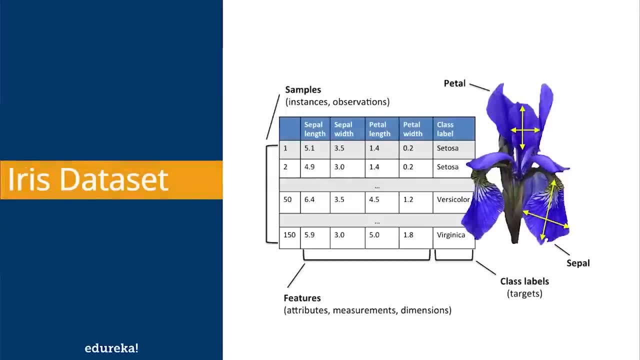 this is the reason why KNN is often referred to as lazy learning algorithm. So this was all about the theoretical session. Now let's move on to the coding part. So for the practical implementation of the hands-on part, I'll be using the IDIS data set. 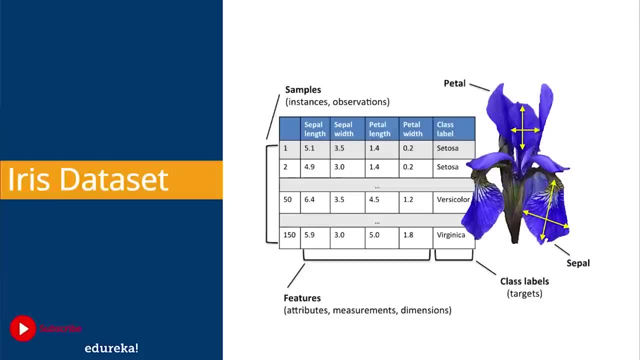 So this data set consists of 150 observation. We have four features and one class label. The four features include the sepal length, the sepal width, petal length and the petal width, Whereas the class label decides which flower belongs to which category. 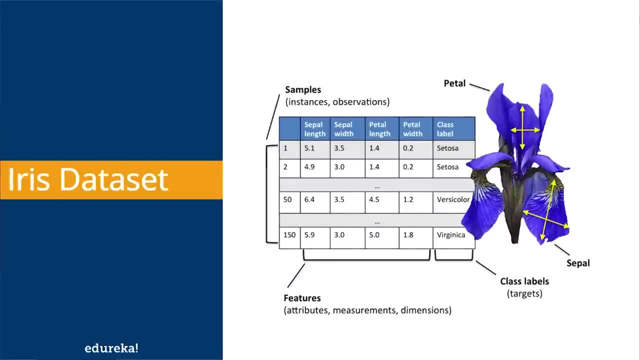 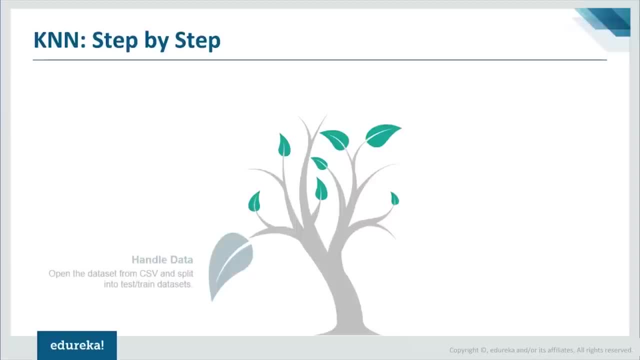 So this was the description of the data set which we are using. Now let's move on and see what are the step-by-step solution to perform a KNN algorithm. So first we'll start by handling the data. What we have to do? we have to open the data set. 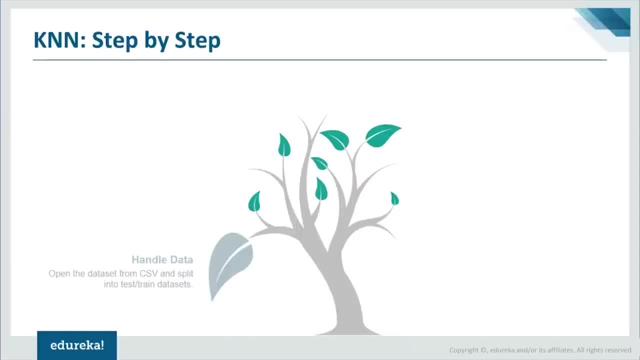 from the CSV format and split the data set into train and test part. Next we'll check the similarity where we have to calculate the distance between two data instances. Once we calculate the distance, next we'll look for the neighbor and select K neighbors. 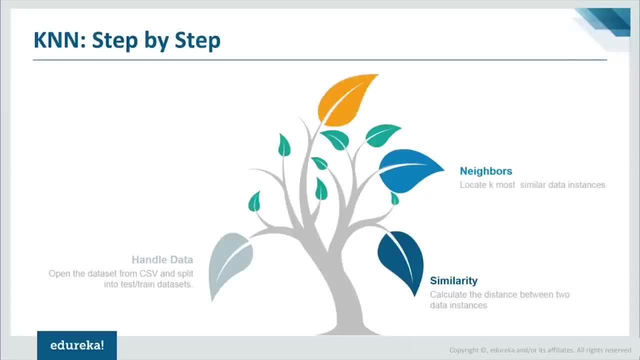 which are having the least distance from a new point. Now, once we get our neighbor, then we'll generate a response from a set of data instances. So this will decide which new point belongs to class A or class B. Finally, we'll create the accuracy function. 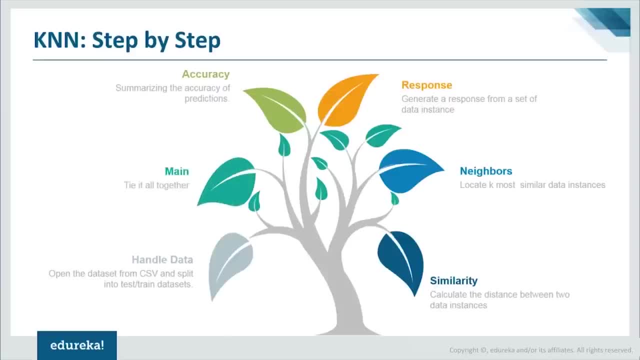 and in the end we'll tie it all together in the main function. So let's start with our code For implementing KNN algorithm using Python. I'll be using Jupyter Notebook, Python 3.0 installed on it. Now let's move on and see how KNN algorithm 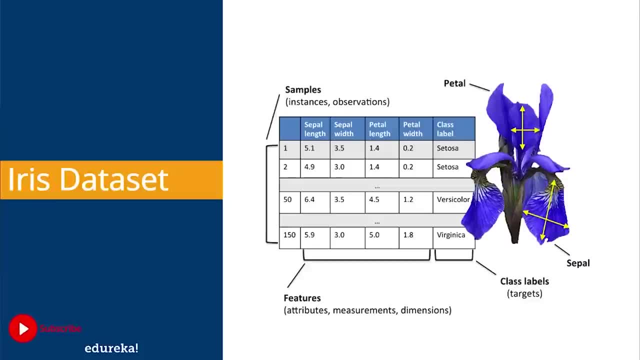 We have four features and one class label. the four features include the sepal length, sepal width, petal length and the petal width, whereas the class label decides which flower belongs to which category. So this was the description of the data set which we are using. 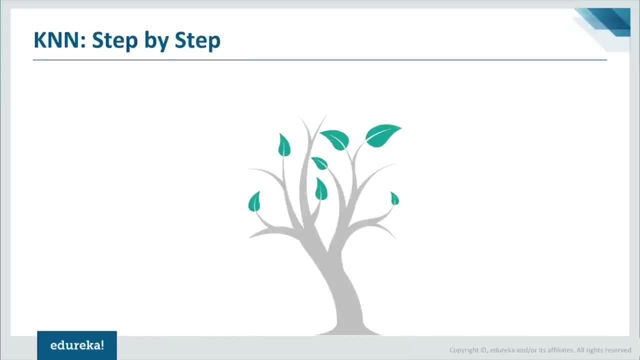 now Let's move on and see what are the step-by-step solution to perform a KNN algorithm. So first we'll start by handling the data. What we have to do? We have to open the data set from the CSV format and split. 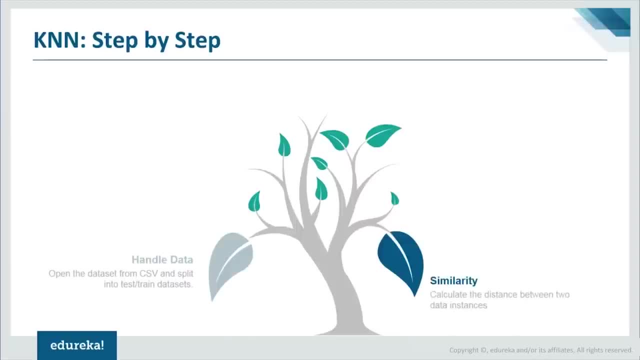 the data set into train and test part. Next We'll check the similarity where we have to calculate the distance between two data instances. Once we calculate the distance, next we'll look for the neighbor and select K neighbors which are having the least distance from a new point. 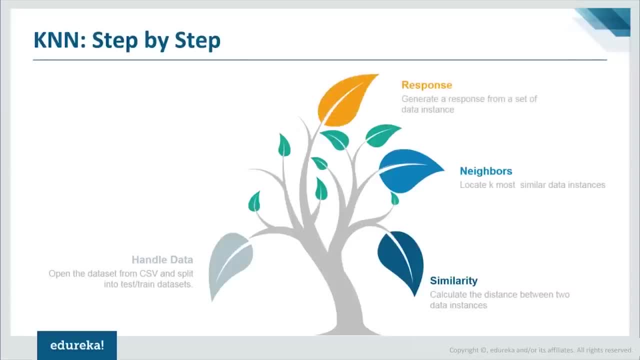 Now, once we get our neighbor, then we'll generate a response from a set of data instances. So this will decide whether the new point belongs to class a or class B. Finally, we'll create the accuracy function and in the end will tie it all together in the main function. 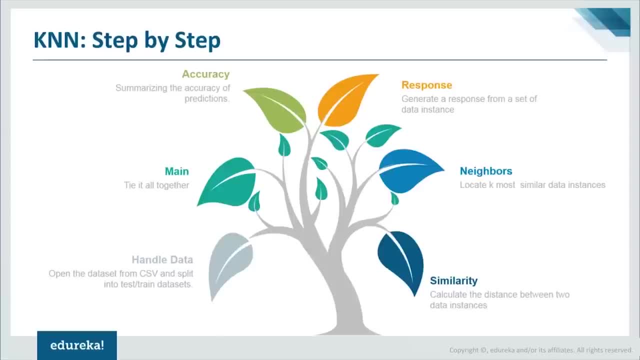 So let's start with our code for implementing KNN algorithm using python. I'll be using Jupiter notebook, python 3.0 install on it. Now let's move on and see how KNN algorithm can be implemented using python. So there's my Jupiter notebook, which is a web-based interactive 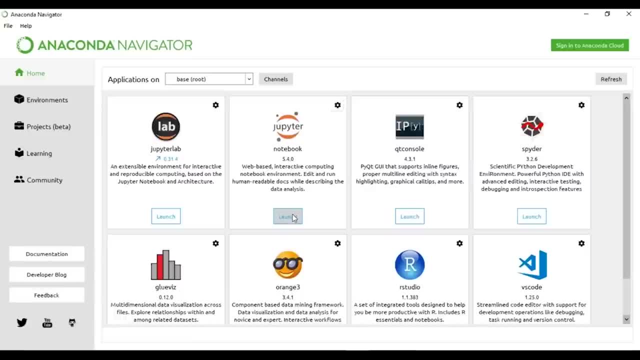 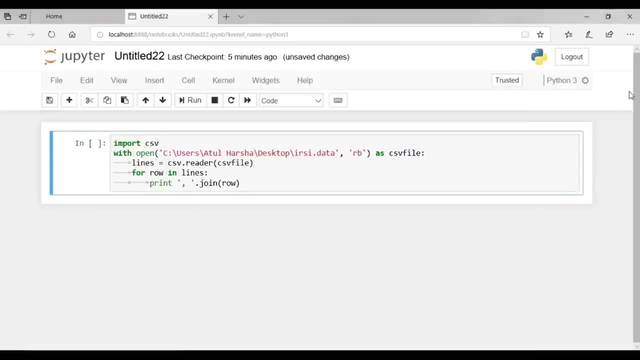 computing notebook environment with python 3.0 installed on it. So the launch? yeah, it's launching. So there's our Jupiter notebook and we'll be writing our python codes on it. So the first thing that we need to do is load our file. 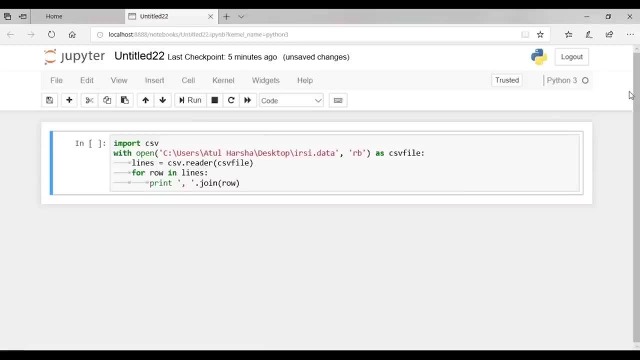 Our data is in CSV format without a header line or any code. We can open the file, the open function, and read the data line using the reader function in the CSV module. So let's write a code to load our data file. Let's execute the run button. 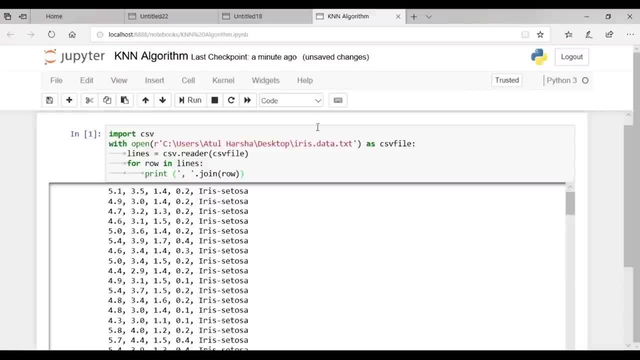 So once you execute the run button, you can see the entire training data set as the output. Next we need to split the data into a training data set that KNN can use to make prediction and a test data set that we can use to evaluate the accuracy of the model. 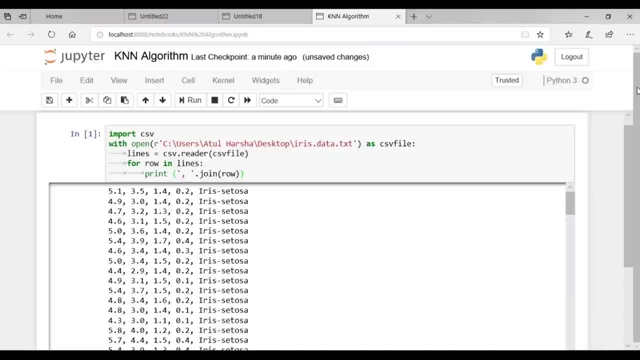 So we first need to convert the flower measure that were loaded as string into numbers that we can work. next We need to split the data set randomly to train and test. a ratio of 67 is to 33 for test is to train as a standard ratio. 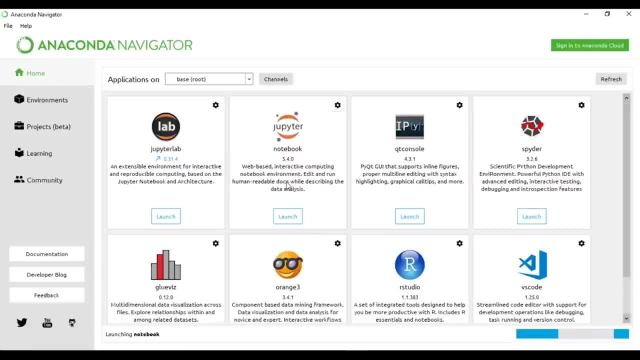 can be implemented using Python. So there's my Jupyter Notebook, which is a web-based interactive computing notebook environment with Python 3.0 installed on it. Set the launch. Yeah, it's launching. So there's our Jupyter Notebook and we'll be writing our Python codes on it. 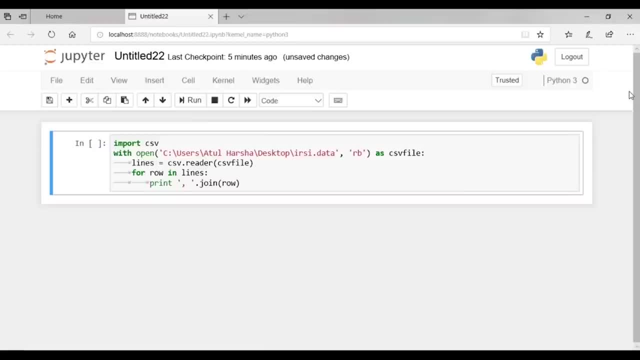 So the first thing that we need to do is load our file. Our data is in CSV format without a header line or any code. We can open the file, the open function, and read the data line using the reader function in the CSV module. 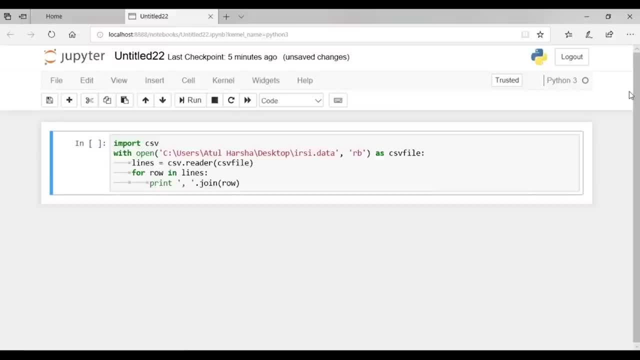 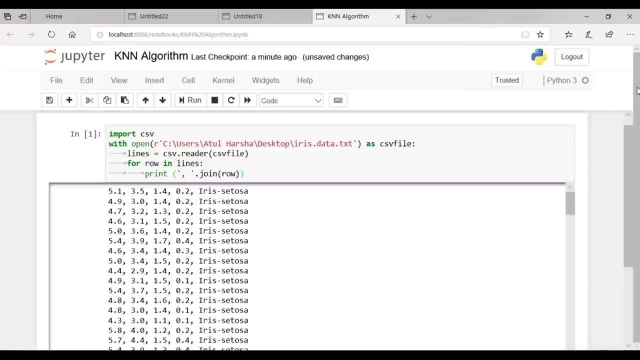 So let's write a code to load our data file. Let's execute the run button. So once you execute the run button, you can see the entire training data set as the output. Next we need to split the data into a training data set. 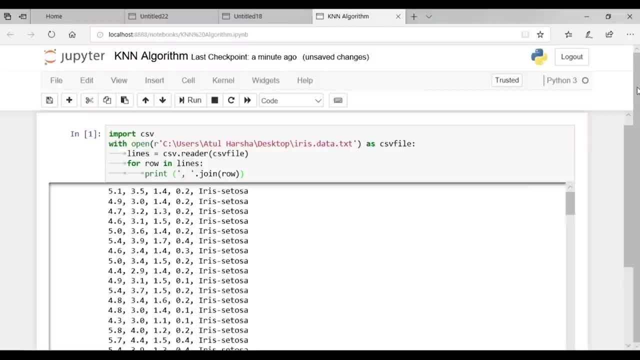 that KNN can use to make prediction and a test data set that we can use to evaluate the accuracy of the model. So we first need to convert the flower measure that were loaded as string into numbers that we can work. Next we need to split the data set randomly to train and test. 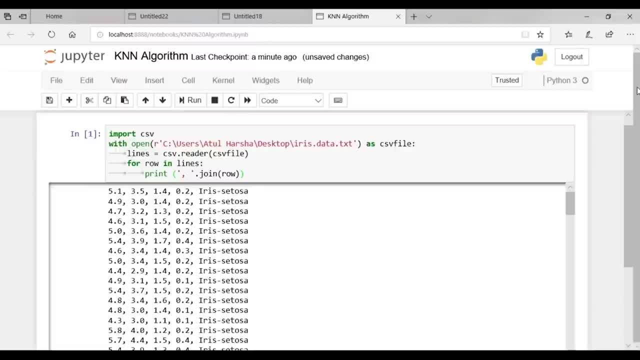 A ratio of 67 is to 33 for test is to train is a standard ratio which is used for this purpose. So let's define a function as load data set that loads a CSV with a provided file name and split it randomly into training and test data set using the provided split ratio. 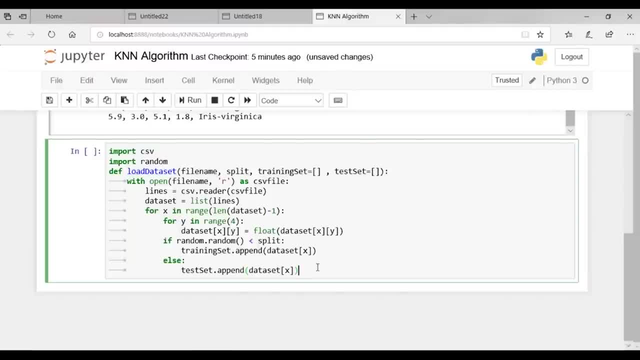 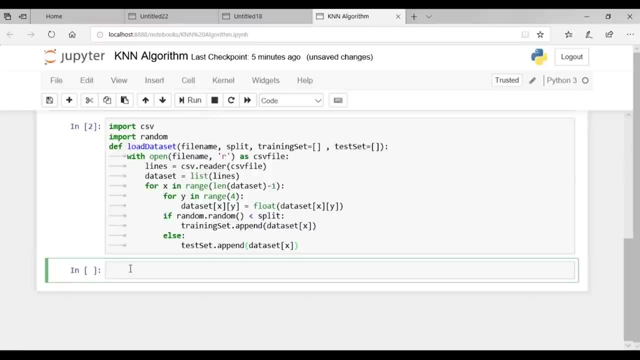 So there's our function load data set, which is using file name, split ratio, training data set and testing data set as its input. All right, so let's execute the run button and check for any errors. So it's executed with zero errors. Let's test this function. 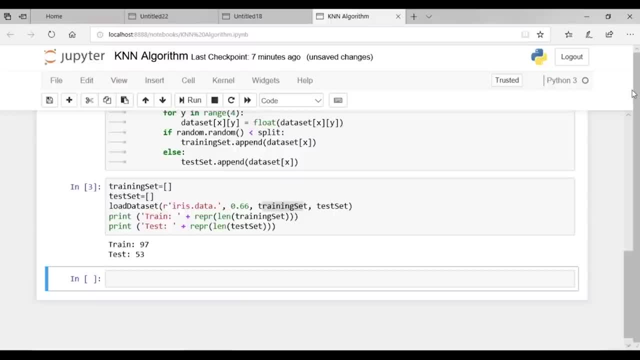 So there's our training set, testing set, load data set. So this is our function- load data set- and inside that we are passing our file, iris data with a split ratio of 0.66, and training data set and test data set. Let's see what our training data set. 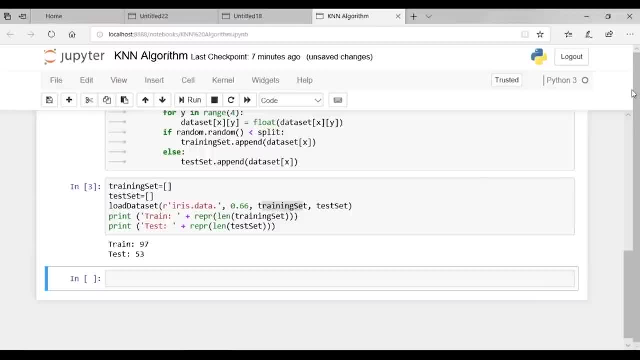 and test data set it's dividing into. So it's giving a count of training data set and testing data set. the total number of training data set it has split into is 97 and total number of test data set we have is 53.. So total number of training data set we have here is 97. 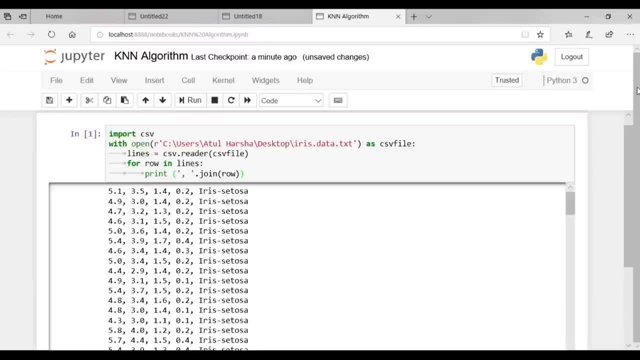 which is used for this purpose. So let's define a function as load data set that loads a CSV with a provided file name and split it randomly into training and test data set using the provided split ratio. So this is our function: load data set, which is using file name. 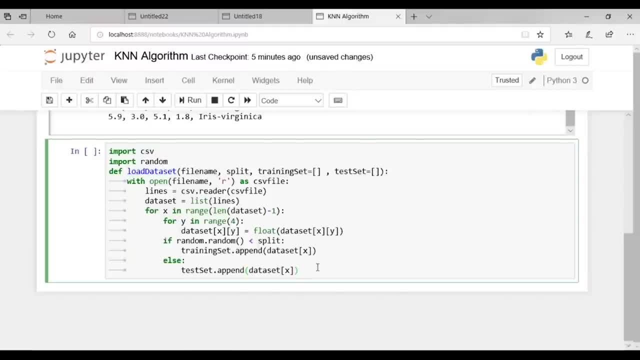 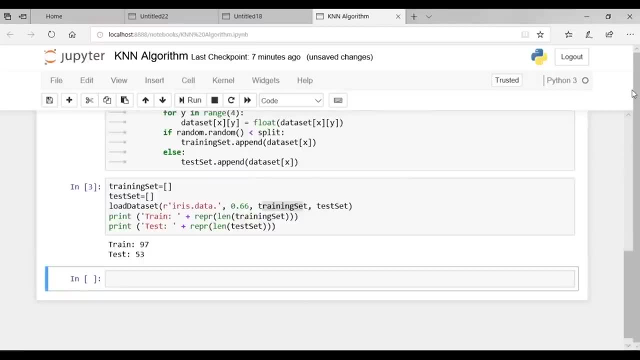 split ratio: training data set and testing data set as its input. All right, so let's execute the run button and check for any errors. So it's executed with zero errors. Let's test this function. So this is our training set testing set. load data set. 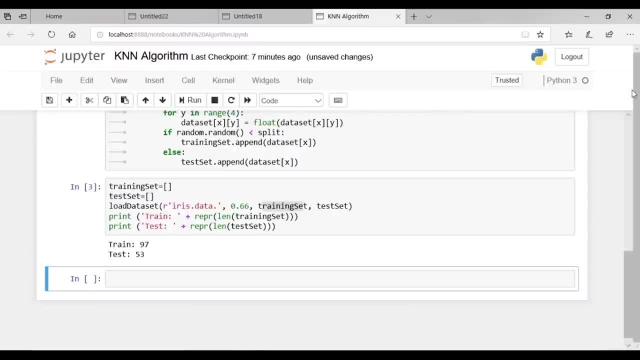 So this is our function: load data set- and inside that we are passing our file, iris data with a split ratio of 0.66 and training data set and test data set. Let's see what our training data set and test data set It's dividing into. just giving a count of training data set. 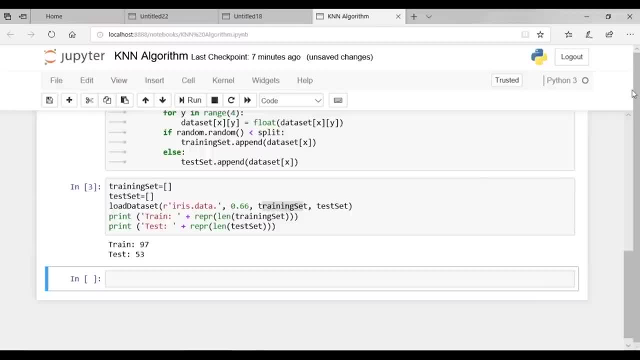 and testing data set. the total number of training data set that has split into is 97 and total number of test data set We have is 53. so total number of training data set We have here is 97 and total number of test data set. 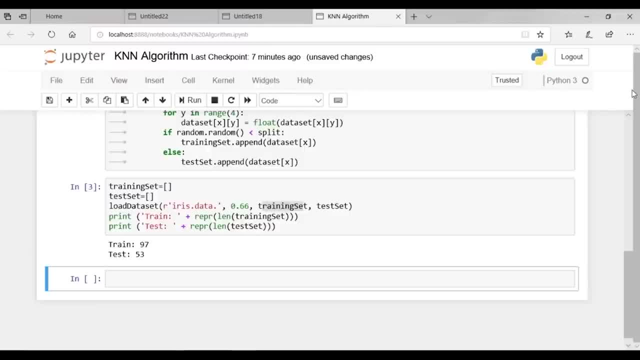 We have here is 53.. All right, Okay, so our function, load data set, is performing well. So let's move ahead to step 2, which is similarity. So, in order to make prediction, we need to calculate the similarity between any two given data instances. this is needed so that 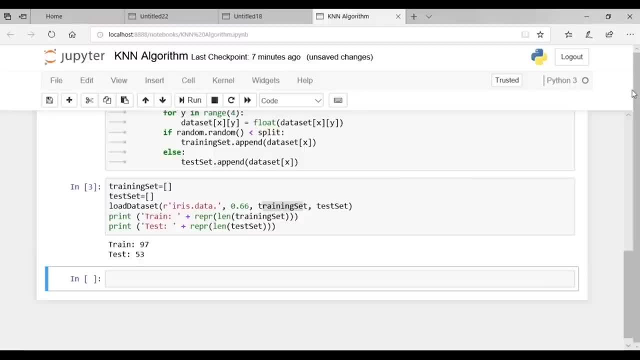 we can locate the K more similar data instances in the training data set and in turn make a prediction. given that all four flower measurement are numeric and have same unit We can directly use, the Euclidean distance measure is nothing but the square root of the sum of squared differences between: 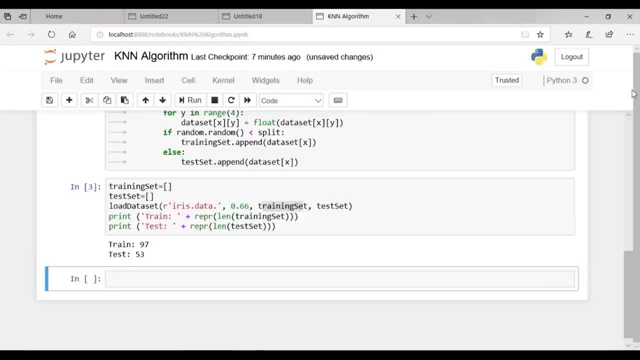 two arrays of the number. given that all the four flower measurements are numeric and have same unit, We can directly use the Euclidean distance measure, which is nothing but the square root of the sum of squared difference between two arrays of the number. Additionally, we want to control which field to include in the 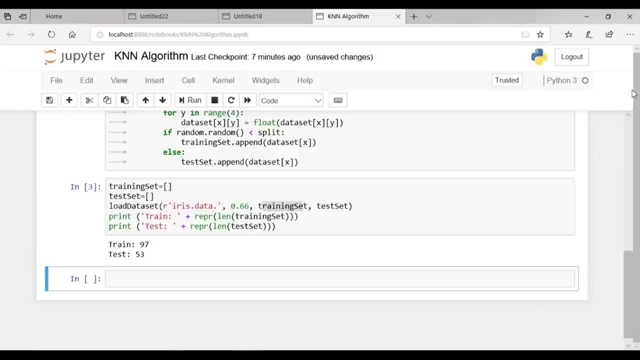 distance calculation. So specifically, we only want to include first four attribute. So our approach will be to limit the Euclidean distance to a fixed length. All right, so let's Define our Euclidean function. So this is our Euclidean distance function, which takes instance. 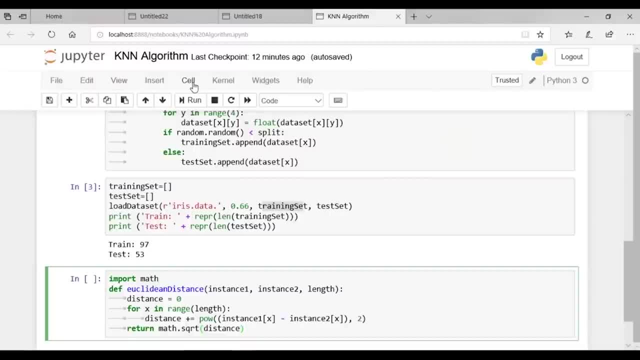 one, instance two and length as parameters. instance one and instance two are the two points of which you want to calculate the Euclidean distance, Whereas this length- and they know that- how many attributes you want to include? Okay, so there's our Euclidean function. 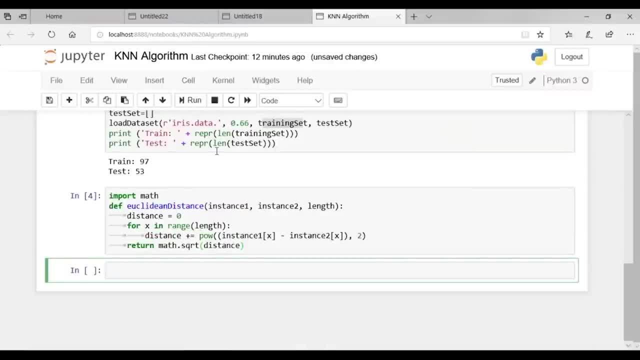 Let's execute it. It's executing fine without any errors. Let's test the function. suppose the data one or the first instance consists of data point as 2, 2, 2, and it belongs to class a, and data to consist of 4, 4, 4, and it belongs to class B. 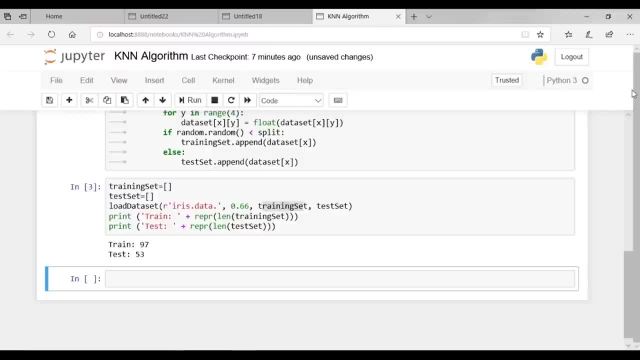 and total number of test data set we have here is 53.. All right, Okay, so our function- load data set- is performing well, So let's move ahead to step 2, which is similarity. So in order to make prediction, we need to calculate. 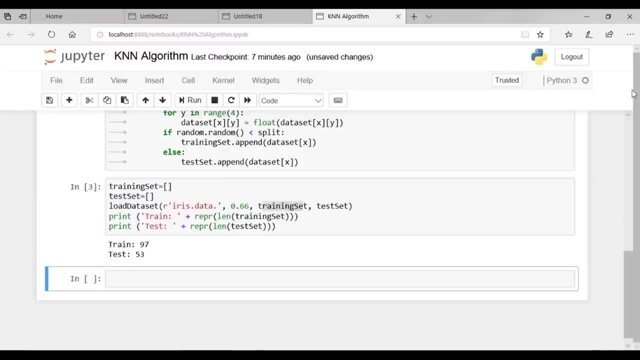 the similarity between any two given data instances. This is needed so that we can locate the K most similar data instances in the training data set and in turn make a prediction. given that all four flower measurement are numeric and have same unit, We can directly use the Euclidean distance measure is nothing. 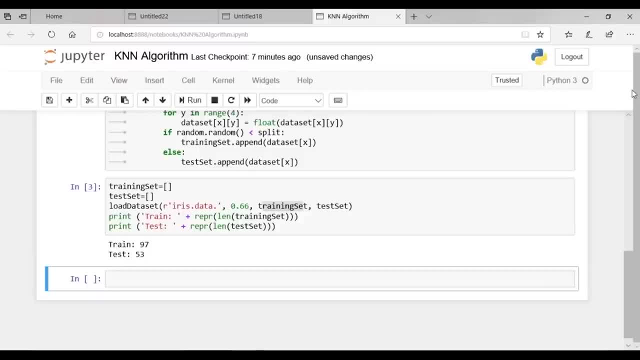 but the square root of the sum of squared differences between two arrays of the number. given that all the four flower measurements are numeric and our same unit, we can directly use the Euclidean distance measure, which is nothing but the square root of the sum of squared difference between two arrays of the number. 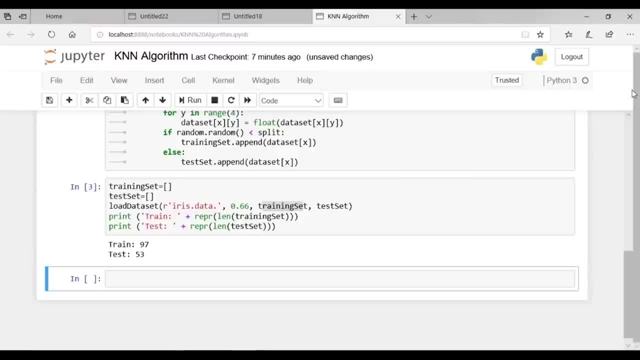 Additionally, we want to control which field to include in the distance calculation. So specifically, we only want to include first four attributes. sort of approach be to limit the euclidean distance to a fixed length. all right, so let's define our euclidean function. so this is our euclidean distance function, which takes instance one instance. 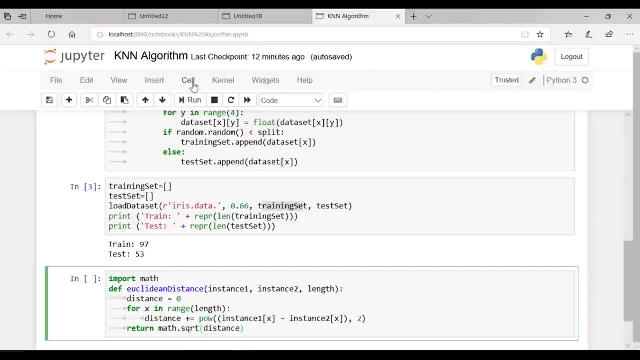 two and length as parameters. instance one and instance two are the two points of which you want to calculate the euclidean distance, whereas this length, and denote that how many attributes you want to include. okay, so there's our euclidean function. let's execute it. it's executing, fine. 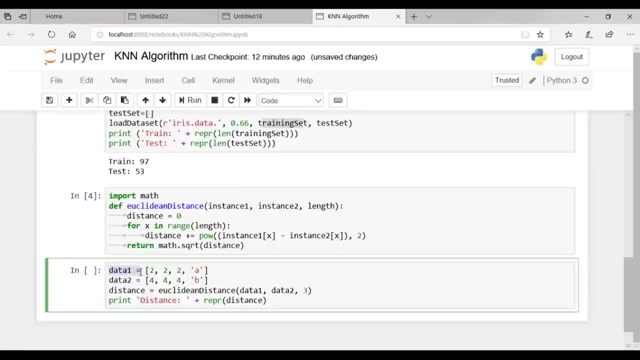 without any errors. let's test the function. suppose the data 1, or the first instance, consists of data point as 2, 2, 2, and it belongs to class a, and data 2 consists of 4, 4, 4, and it belongs to class b. so when we calculate the euclidean distance of data 1 to data 2 and what we have to do, we have: 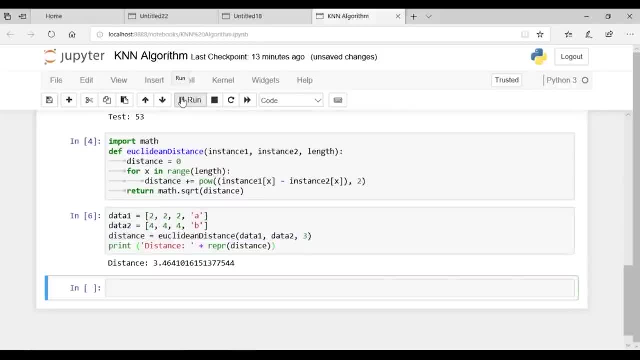 to consider only first three features of them. all right, so let's print the distance. as you can see here, the distance comes out to be 3.464. all right, so this is nothing but the square root of 4 minus 2 whole square. so this distance is nothing but. 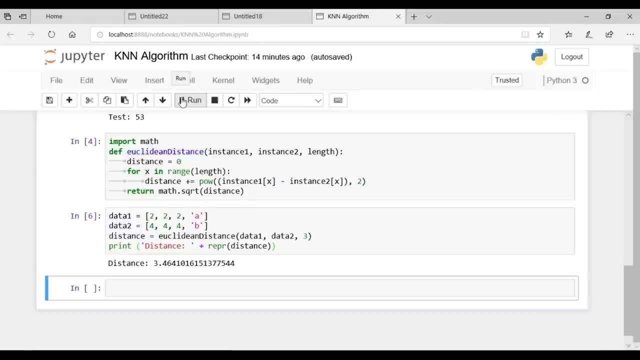 4 minus 2 whole square, so this distance is nothing but 4 minus 2 whole square. so this distance is nothing but the euclidean distance and it is calculated as square root of 4 minus 2 whole square. plus 4 minus 2 whole square, that is nothing but 3 times of 4 minus 2 whole square, that is 12 and square root. 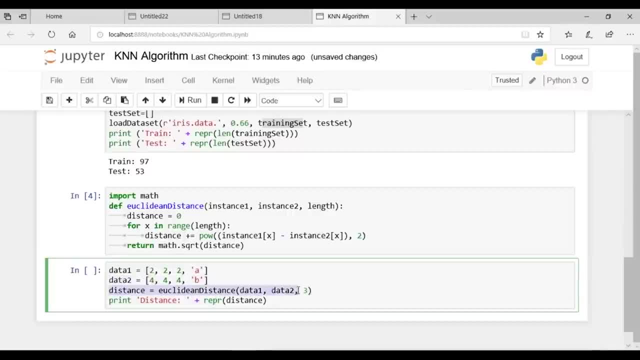 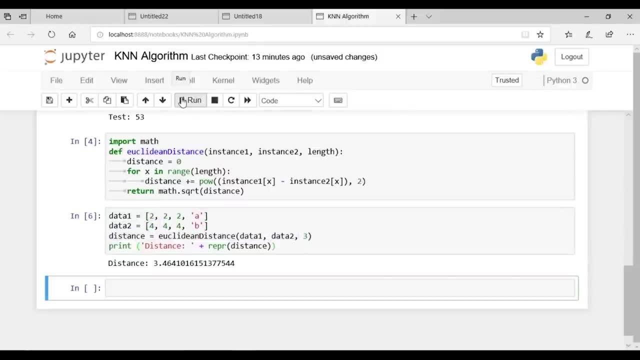 So when we calculate the Euclidean distance of data 1 to data 2, and what we have to do, we have to consider only first three features of them. All right, so let's print the distance. as you can see here, the distance comes out to be 3.464.. 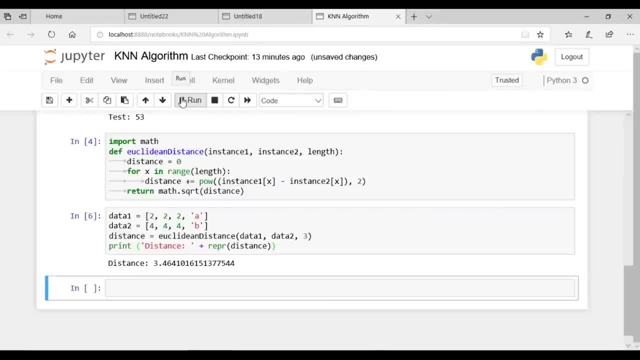 All right. so this is nothing but the square root of 4 minus 2 whole square. So this distance is nothing but the Euclidean distance and it is calculated as square root of 4 minus 2 whole square. plus 4 minus 2 whole square, that is nothing but 3 times of 4 minus. 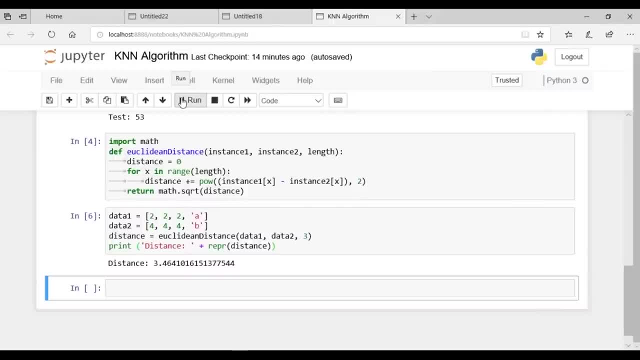 2. whole square, that is 12, and square root of 12 is nothing but 3.464.. All right, So now that we have calculated the distance, now we need to look for K nearest neighbors. now that we have a similarity measure, we can use it to collect the K most similar instances. 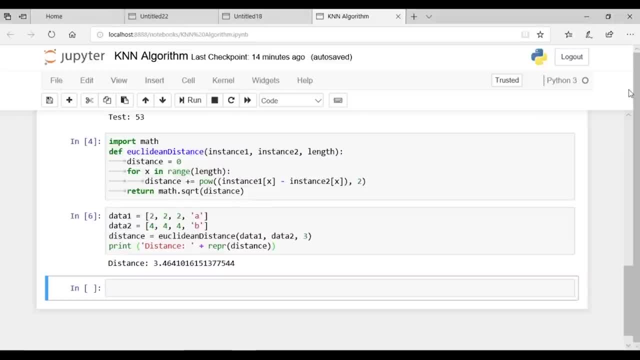 for a given unseen instance. Well, this is a straightforward process of calculating the distance for all the instances and selecting a separate subset with a smallest distance value. and now what we have to do? We have to select the smallest distance values. So for that will be defining a function as get neighbors. 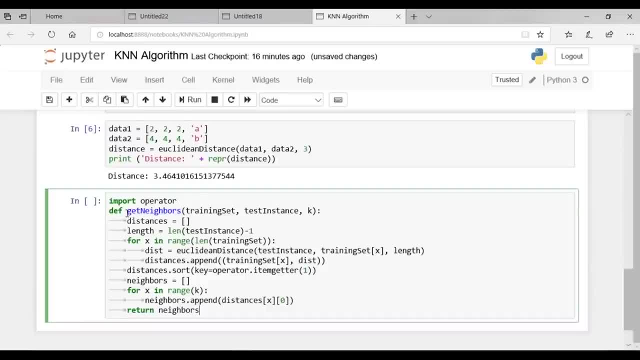 So for that, what we'll be doing will be defining a function as get neighbors. what it will do, it will return the K most similar neighbors from the training set for a given test instance. All right, So this is how our get neighbors function. look like it takes. 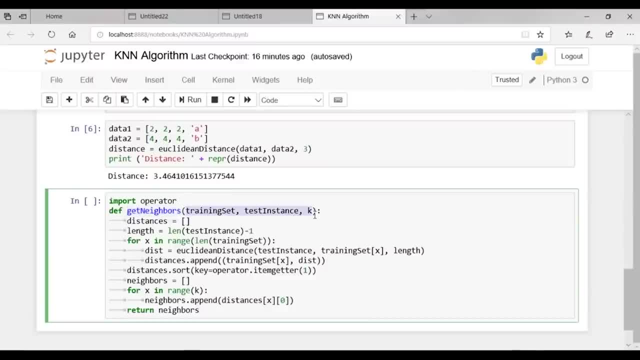 training data set and test instance and K as its input. here the K is nothing but the number of nearest neighbor you want to check for. All right, So basically, what you will be getting from this Get neighbors function is K, different points having least Euclidean distance from the test instance. 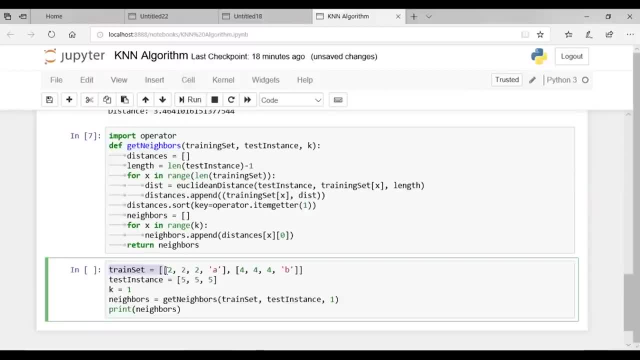 All right, let's execute it. So the function executed without any errors. So let's test our function. So suppose the training data set includes the data like 2, 2, 2 and it belongs to Class A, and other data includes 4, 4, 4 and. 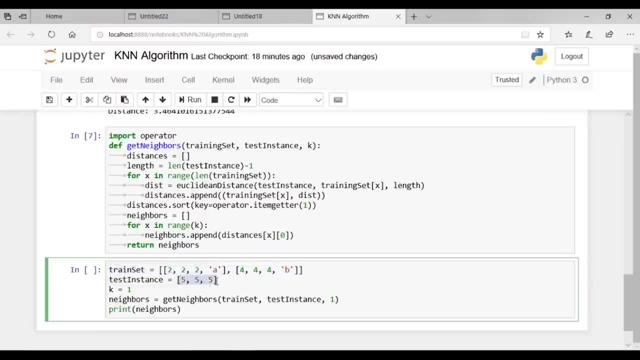 it belongs to Class B and our testing instances 5, 5, 5 or now we have to predict whether this test instance belongs to Class A or it belongs to Class B. All right, for K equal 1, we have to predict its nearest neighbor and predict whether this test instance it will belong to Class 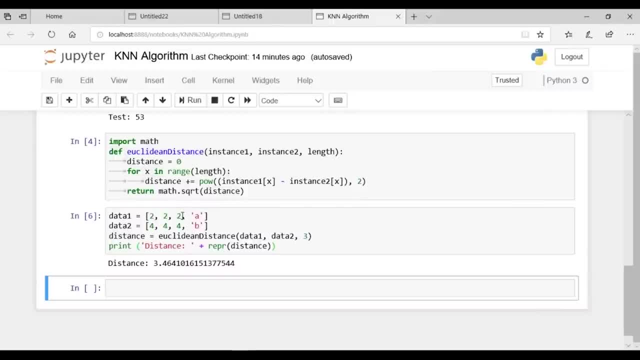 of 12 is nothing but 3.464. all right, so now that we have calculated the distance, now we need to look for k nearest neighbors. now that we have a similarity measure, we can use it to collect the k most similar instances for a given unseen instance. well, this is a straightforward process of calculating. 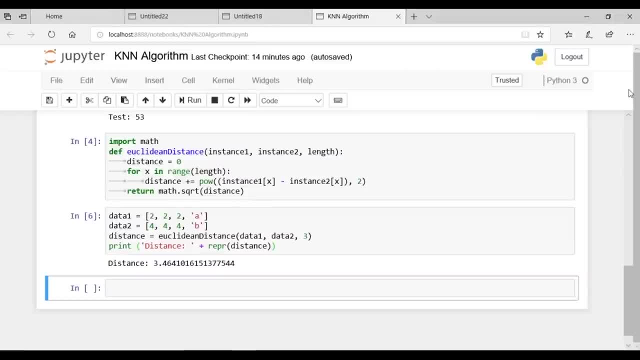 the distance for all the instances and selecting a subset with the smallest distance value. and now what we have to do? we have to select the smallest distance values, so for that we'll be defining a function. as get neighbors. so for that, what we'll be doing, we'll be defining a function. 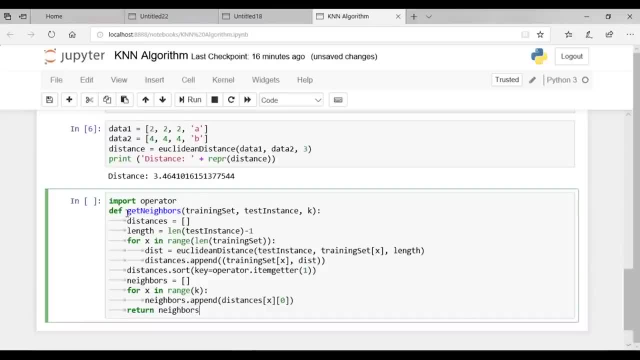 as get neighbors. what it will do? it will return the k most similar neighbors from the training set for a given test instance. all right, so this is how our get neighbors function look like. it takes training data set and test instance and k as its input. here the k is nothing but the number of 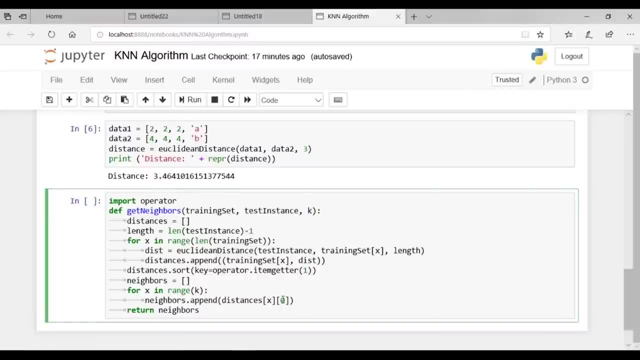 nearest neighbor you want to check for. all right, so basically, what you'll be getting from this get neighbors function is k- different points- and you can see that the k is nothing but the number of points having least euclidean distance from the test instance. all right, let's execute it. so the 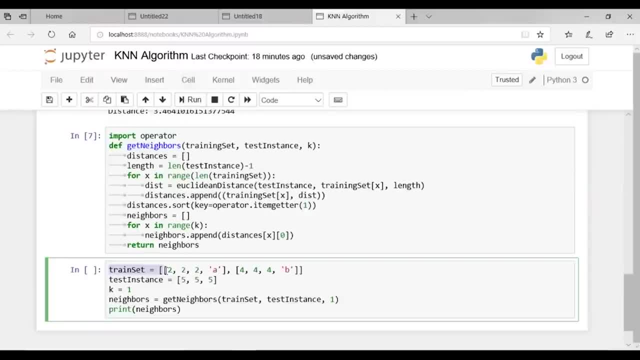 function executed without any errors. so let's test our function. so suppose the training data set includes the data like two, two, two, and it belongs to class a. and other data includes four, four, four, and it belongs to class b, and our testing instance is five, five, five. and now we have to predict. 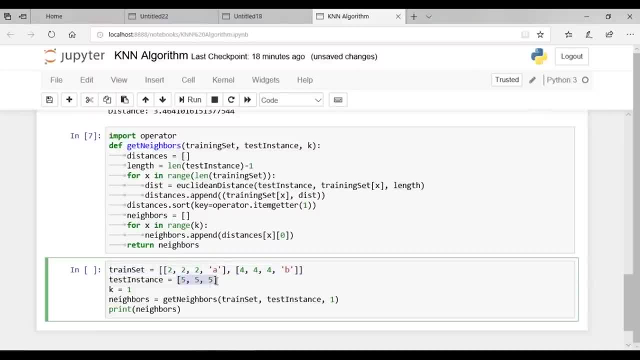 whether this test instance belongs to class a or it belongs to class b. all right, for k equal one, we have to predict its nearest neighbor and predict whether this test instance it will belong to class a or will it belong to class b. all right, so let's execute the run button. all right, so on. 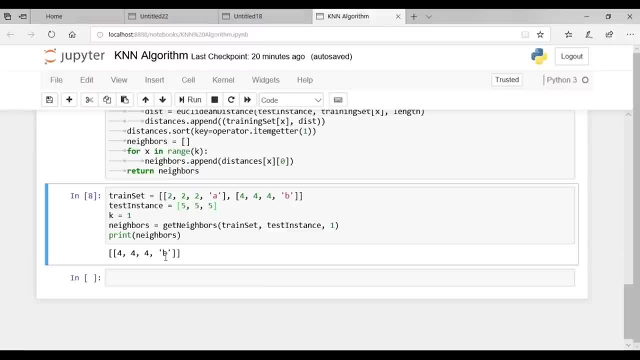 executing the run button, you can see that we have output as four, four, four and b. our new instance, five, five, five, is closest to point four, four, four, which belongs to class b. all right now, once you are located the most similar neighbor for a test instance, next task is to predict a response. 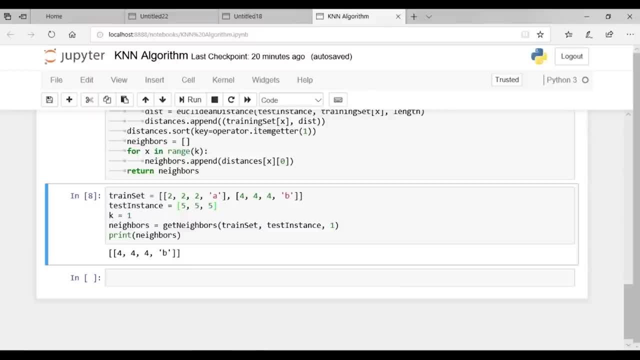 based on those neighbors. so how we can do that? well, we can do this by allowing each neighbor to vote for the class attribute and take the majority vote as a prediction. let's see how we can do that. we have a function as get response, which takes neighbors as the input. well, this neighbor was. 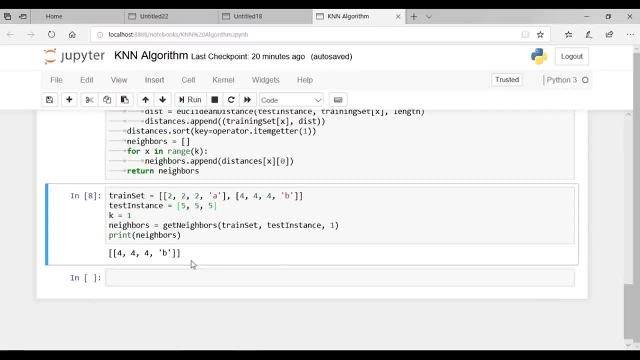 A or will it belong to Class B? All right, so let's execute the run button. All right, So in executing the run button, you can see that we have output as 4, 4, 4 and be our new instance: 5, 5. 5 is closest to point 4, 4. 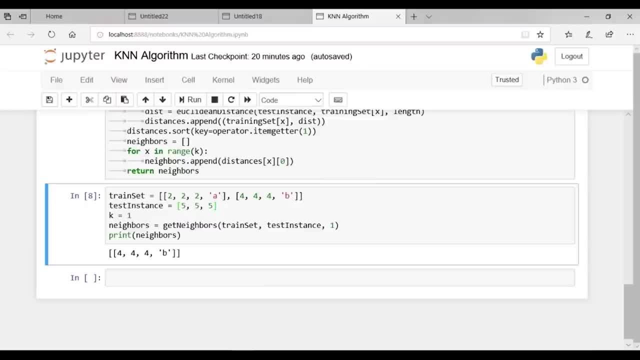 4, which belongs to Class B. All right Now, once you are located the most similar neighbor for a test instance, next task is to predict a response based on those neighbors. So how we can do that? Well, we can do this by allowing each neighbor to vote for the. 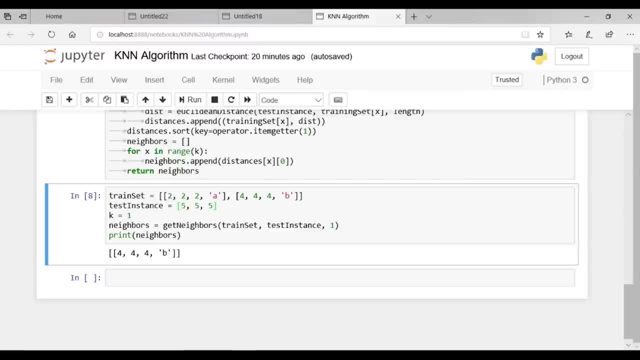 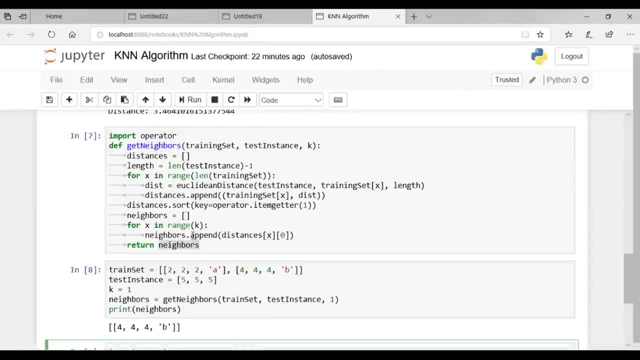 class attribute and take the majority vote as the percentage prediction. Let's see how we can do that. So we have a function as get response which takes neighbors as the input. Well, this neighbor was nothing but the output of this get neighbor function. 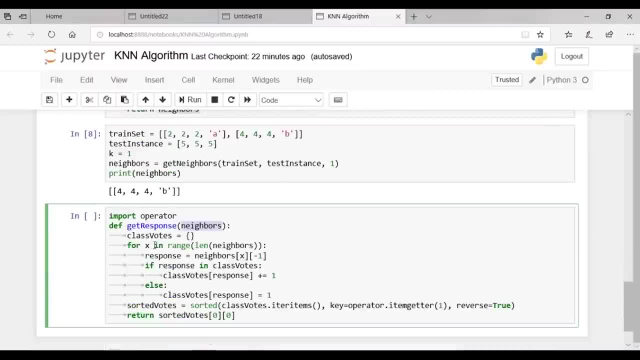 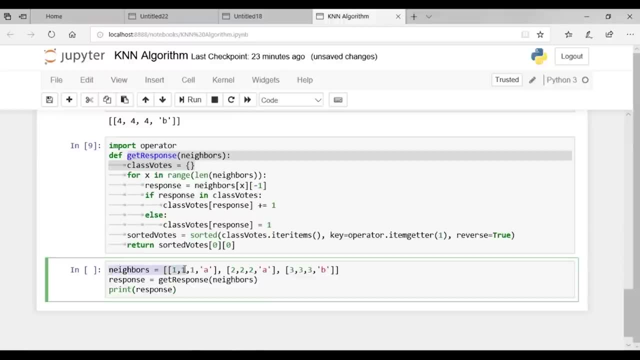 The output of get neighbor function will be fed to get response. All right, let's execute the run button. It's executed, Let's move ahead and test our function. get response. So we have a neighbor as 1, 1, 1. it belongs to Class A, 2, 2, 2 it. 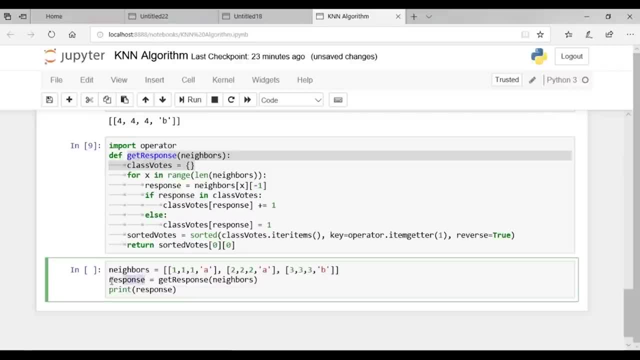 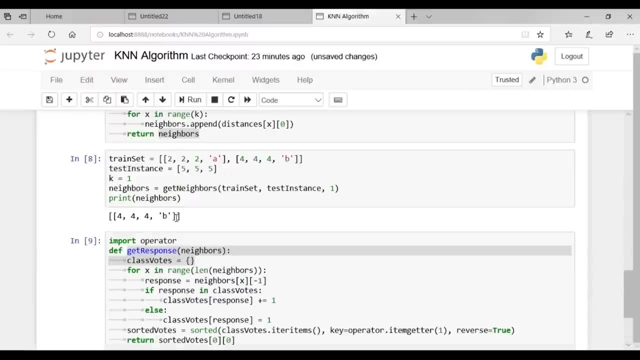 belongs to Class A. 3, 3, 3: it belongs to Class B. So this response, what it will do, will store the value of get response App, bypass This neighbor value, All right. so what we want to check is, we want to predict. 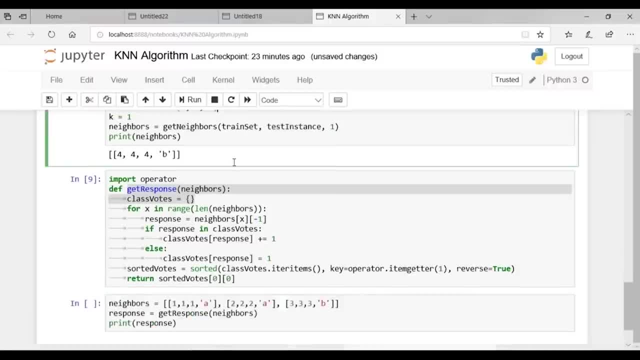 whether that test instance 555, it belongs to Class A or Class B when the neighbors are 1- 1, 1 a, 2, 2, 2 a and 3- 3, 3 B. So let's check our response Now that we have created all the different function, which are: 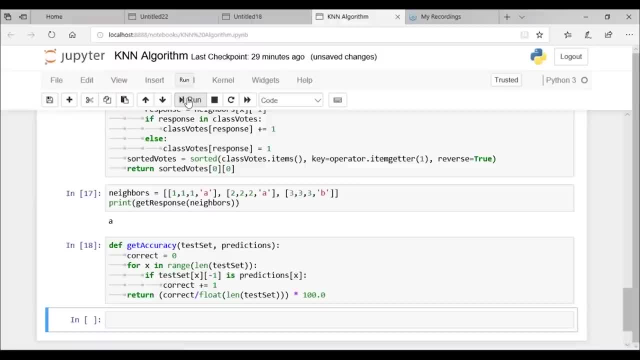 required for a canon algorithm. So important main concern is how to evaluate the accuracy of the prediction. and easy way to evaluate the accuracy of the model is to calculate a ratio of the total correct prediction to all The prediction made. so for this I'll be defining function as 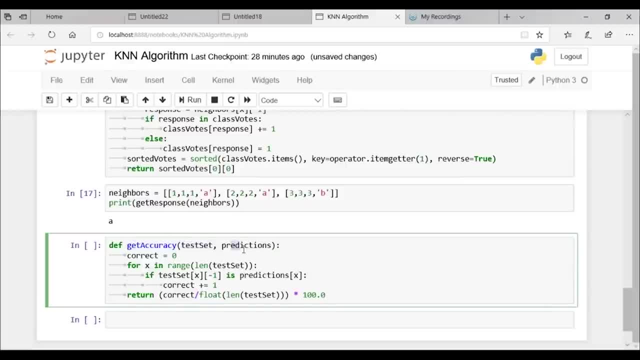 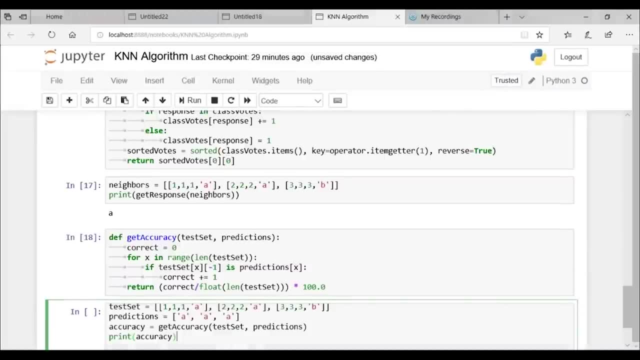 get accuracy and inside that I'll be passing my test data set and the predictions. get accuracy function. check it, execute it without any error. Let's check it for a sample data set. So we have our test data set as 1 1, 1, which belongs to Class A. 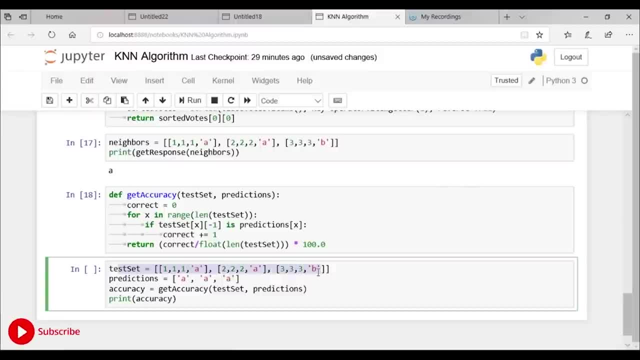 2, 2, 2, which again belongs to Class 3, 3, 3, which belongs to Class B. and my predictions is: for first test data, It predicted that it belongs to Class A, which is true. for next, it predicted that belongs to Class A, which is again true. and 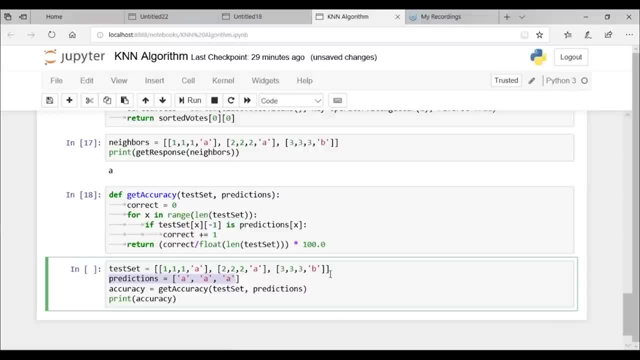 for the next again, and predicted that it belongs to Class A, which is false in this case because the test data belongs to Class B. All right, So in total, we have two correct prediction out of three. All right, So the ratio will be 2 by 3, which is nothing but 66.66. 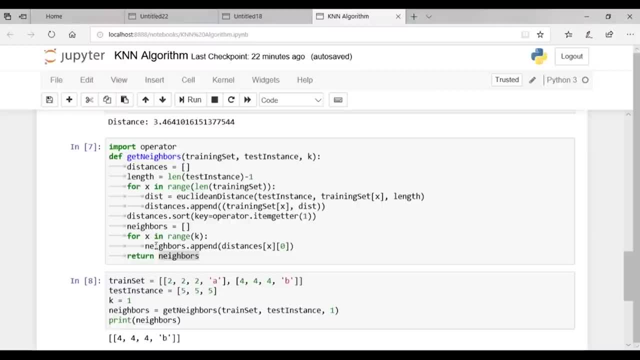 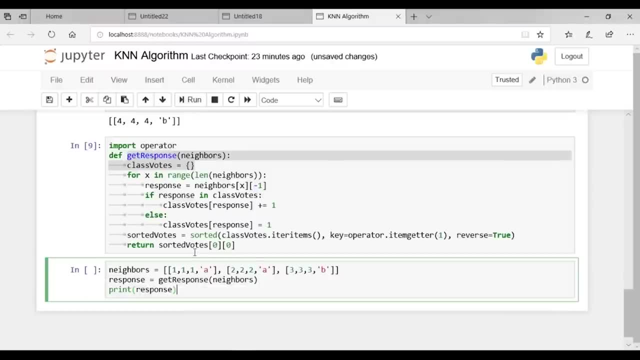 nothing but the output of this get neighbor function. the output of get neighbor function will be fed to get response. all right, let's execute the run button. it's executed. let's move ahead and test our function. get response. so we have a neighbor as one one one. it belongs to class a. 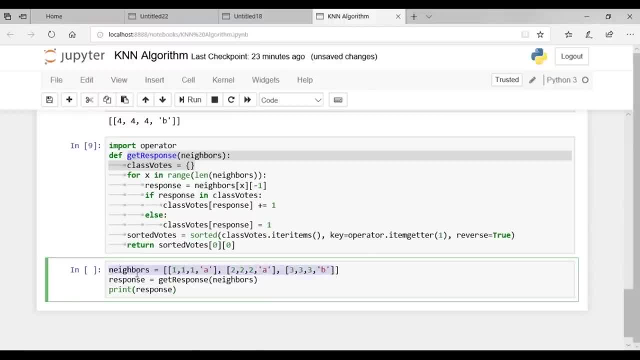 two, two, two. it belongs to class a, three, three, three, it belongs to class b. so this response, what it will do, it will store the value of get response by passing this neighbor value. all right, what we want to check is we want to predict whether our test instance 555 it belongs to. 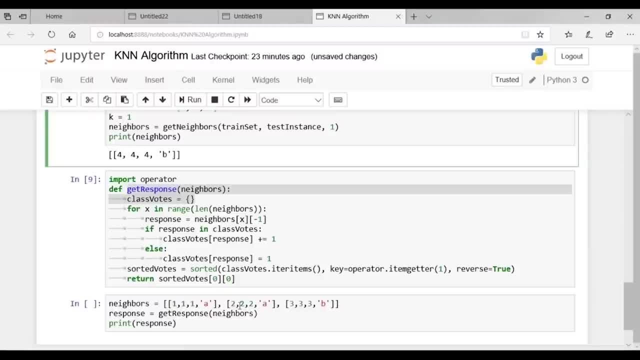 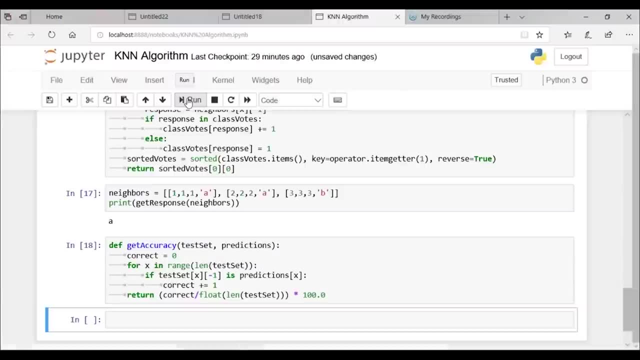 class a or class b when the neighbors are 111 a, 222 a and 333 b. so let's check our response now that we have created all the different function which are required for a canon algorithm. so important main concern is how to evaluate the accuracy of the prediction. an easy way to evaluate. 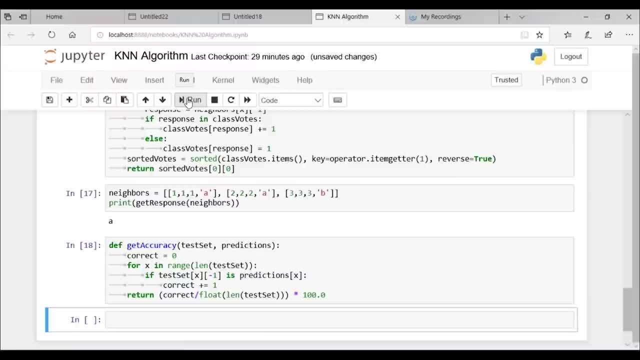 the accuracy of the model is to calculate a ratio of the total correct prediction to all the prediction made. so for this i'll be defining function as get accuracy and inside that i'll be passing my test data set and the predictions. get accuracy function: check it, execute it without. 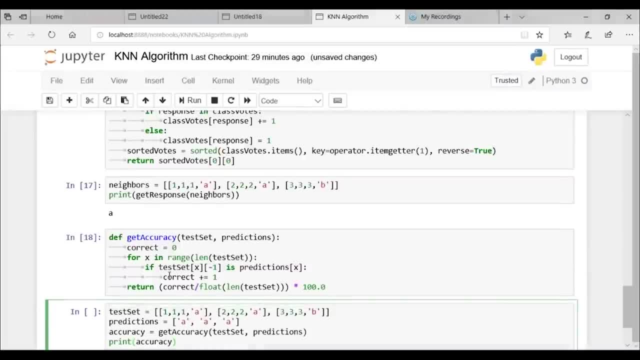 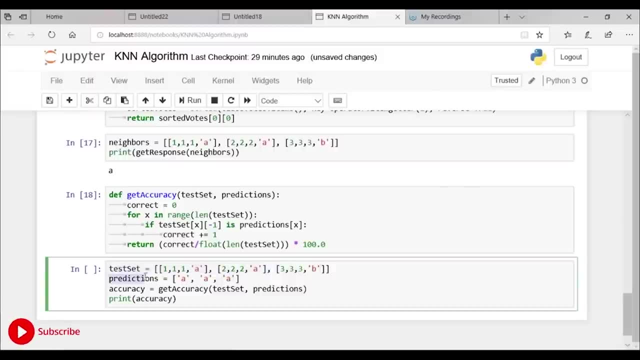 any error, let's check it for a sample data set. so we have our test data set as 111, which belongs to class a, 222, which again belongs to class 333, which belongs to class b, and my predictions is: for first test data, it predicted that it belongs to class a, which is true. for next, it predicted 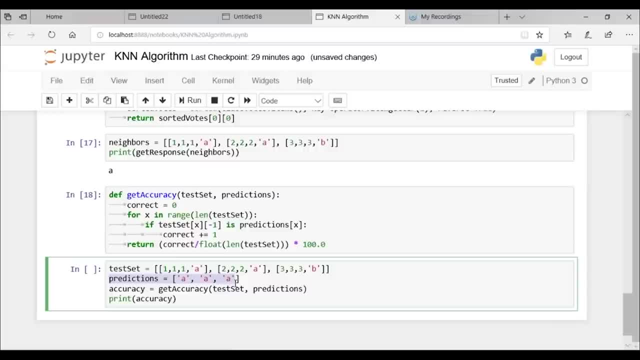 that belongs to class a, which is again true, and for the next, again it predicted that it belongs to class a, which is false in this case because the test data belongs to class b. all right, so in total, we have two correct prediction out of three, all right. 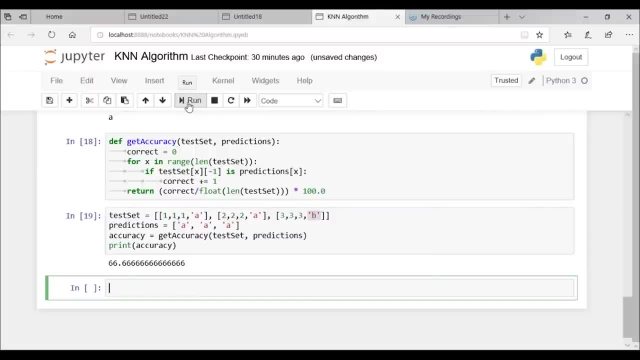 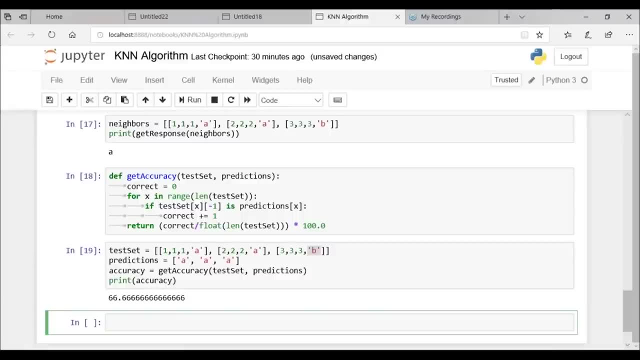 so the ratio will be 2 by 3, which is nothing but 66.66. so our accuracy rate is 66.66. so now that you have created all the function that are required for canon algorithm, let's compile them into one single main function. all right, so this is our main function and we are using iris data. 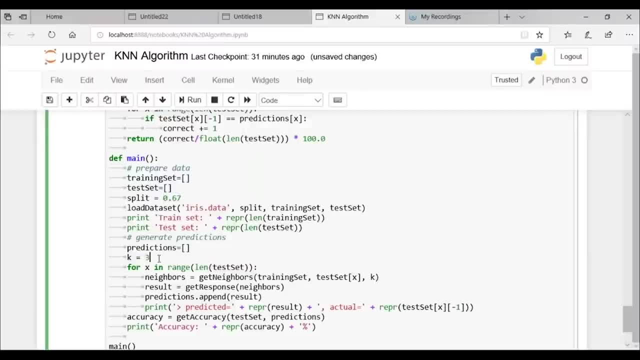 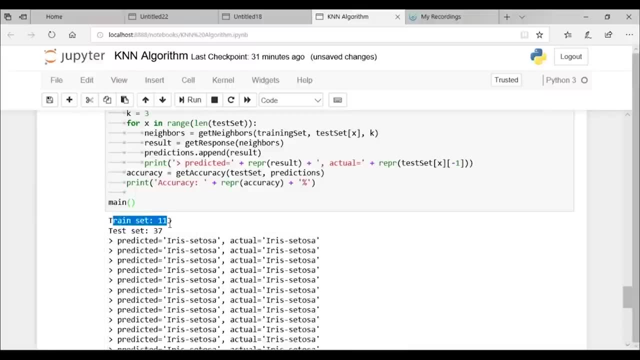 set with a split of 0.67 and the value of k is 3. let's see what is the accuracy score of this. check how accurate our model is. so in training data set we have 113 values and in the test data set we have 37 values. these are the predicted and. 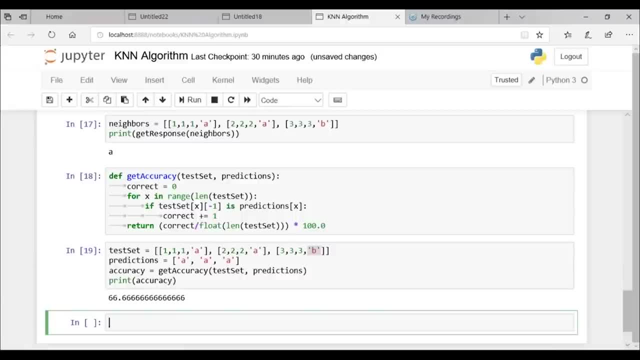 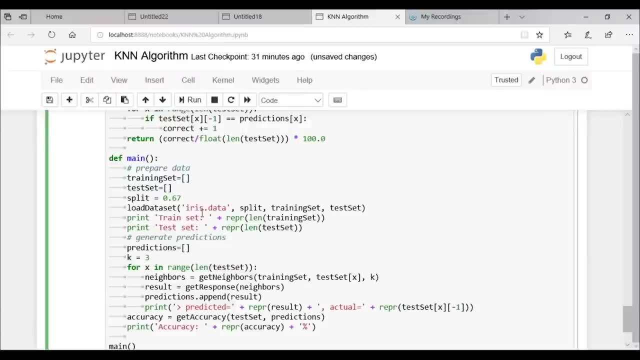 So our accuracy rate is 66.66.. So now that you have created all the function that are required for Canon algorithm, Let's compile them into one single main function. All right, So there's our main function, and we are using Iris data set. 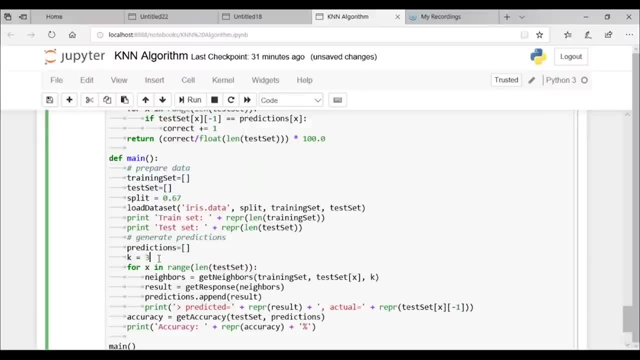 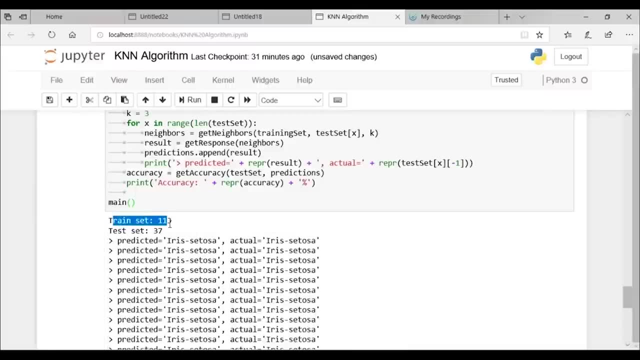 with a split of 0.67 and the value of K Is 3.. Let's see What is the accuracy score of this. check how accurate our model is. So in training data set we have 113 values. and then the test data set. 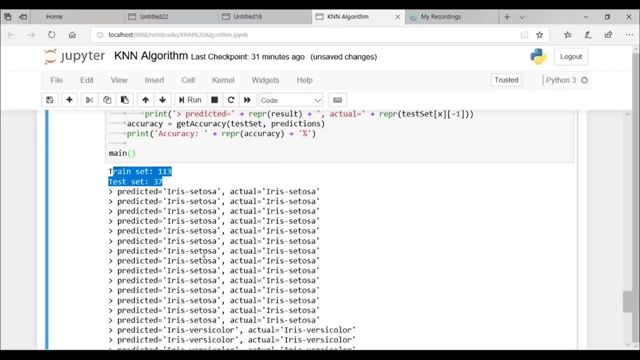 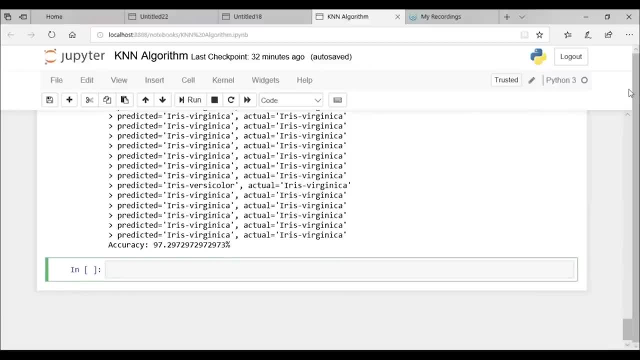 We have 37 values. These are the predicted and the actual values of the output. Okay, So in total we got an accuracy of 97.29%, which is really very good. All right, So I hope the concept of this Canon algorithm is clear to. 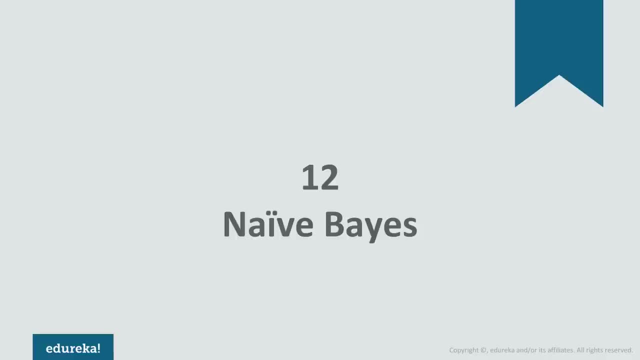 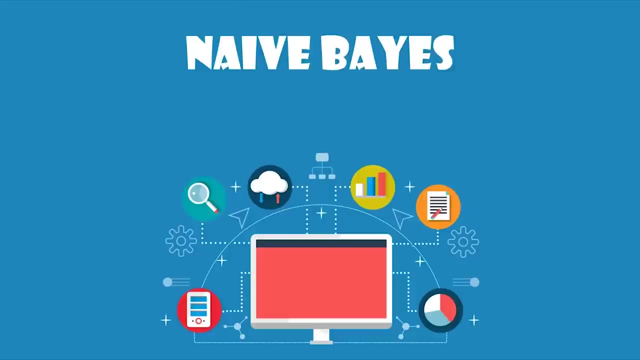 guys, In a world full of machine learning and artificial intelligence surrounding almost everything around us, classification and prediction is one of the most important aspects of machine learning. So, before moving forward, let's have a quick look at the agenda. I'll start off this video by explaining you guys. 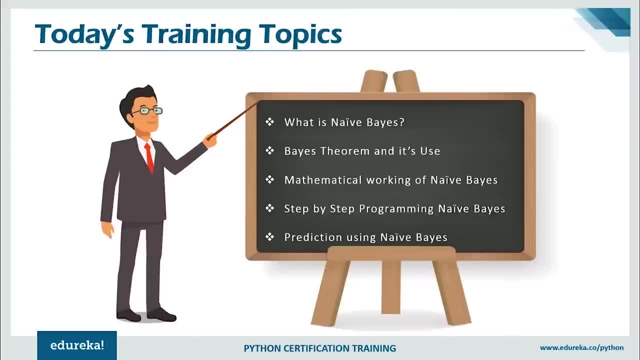 What exactly is naive bias? Then we'll understand what is Bayes theorem, which serves as a logic behind the naive bias algorithm. Moving forward, I'll explain the steps involved in the naive bias algorithm one by one and finally, I'll finish off this video with a. 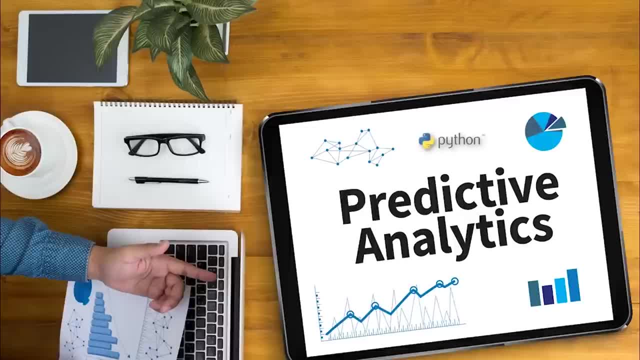 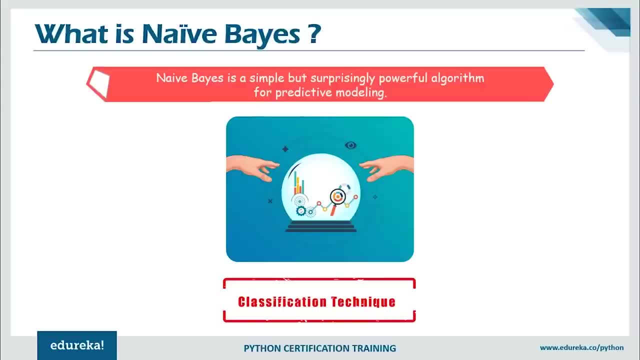 demo on the naive bias Using the sklearn package. Now, naive bias is a simple but surprisingly powerful algorithm from predictive analysis. It is a classification technique based on Bayes theorem with an assumption of Independence among predictors. It comprises of two parts, which is naive and bias. in simple, 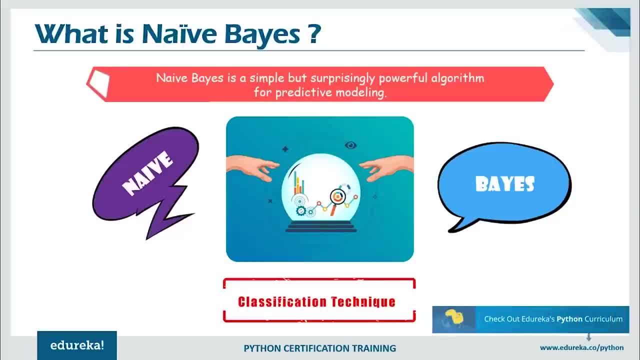 terms. naive bias classifier assumes that the presence of a particular feature in a class is unrelated to the presence of any other feature, even if this features depend on each other or upon the existence of the other features. all of these properties independently contribute to the probability whether a fruit is an. 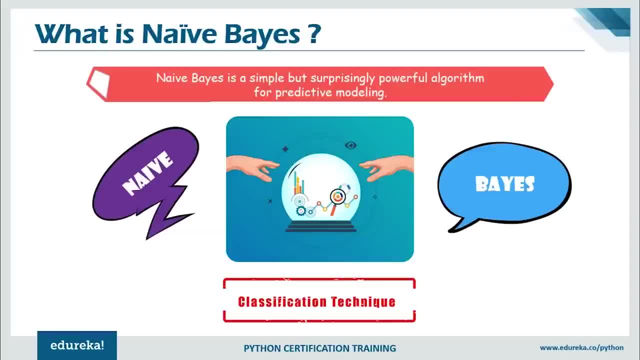 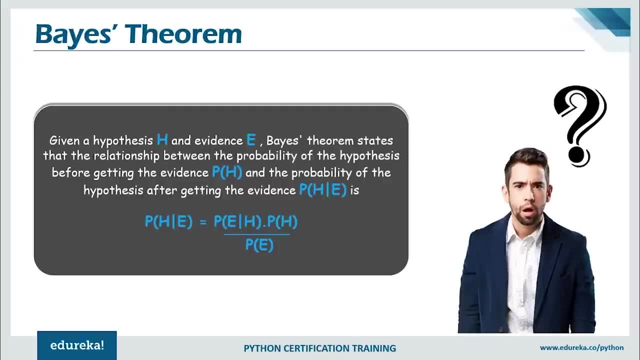 apple or an orange or a banana, So that is why it is known as naive. Now, naive based model is easy to build and particularly useful for very large data sets. in probability Theory and statistics based theorem, which is alternatively known as the Bayes law or the Bayes rule, describes the probability of an event based 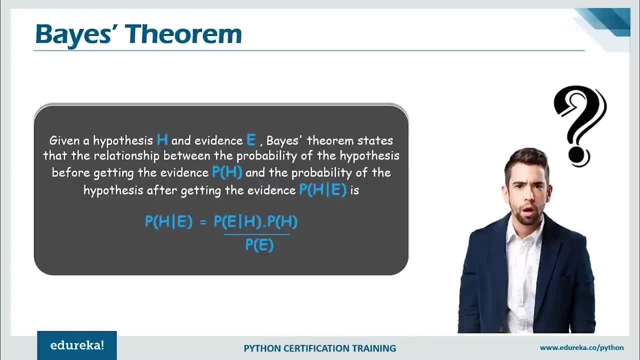 on prior knowledge of the conditions that might be related To the event. now, Bayes theorem is a way to figure out conditional probability. The conditional probability is the probability of an event happening, given that it has some relationship to one or more other events. For example, your probability of getting a parking space is. 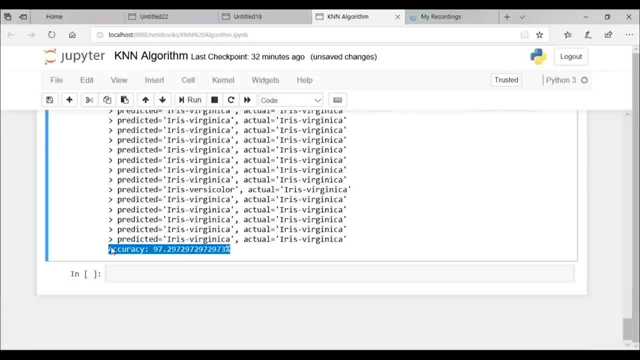 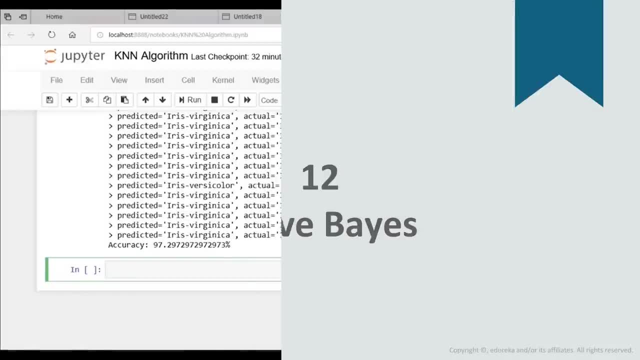 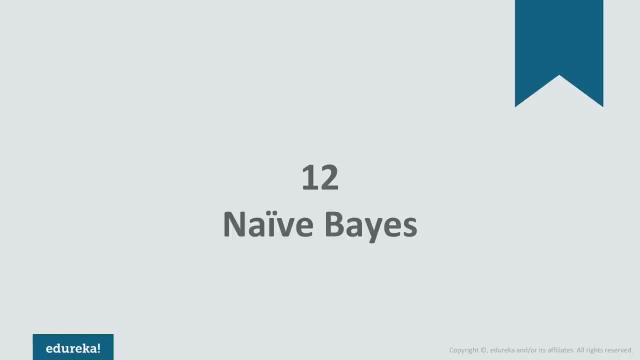 the actual values of the output. okay, so in total we got an accuracy of 97.29, which is really very good. all right, so i hope the concept of this canon algorithm is clear to you guys. in a world full of machine learning and artificial intelligence surrounding almost everything around us, classification and prediction is one of the most. 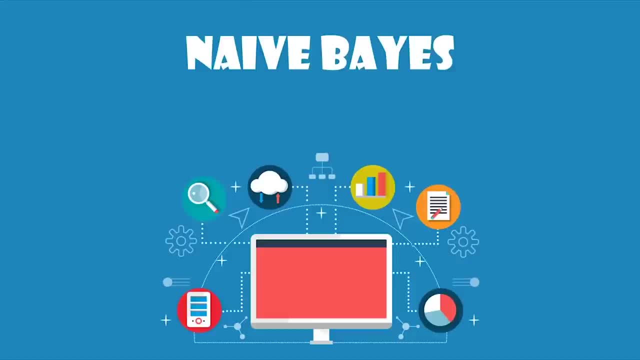 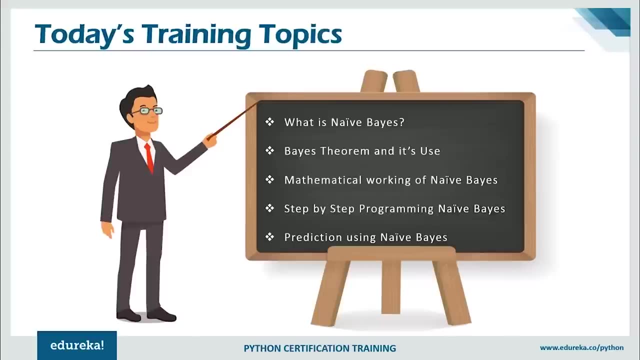 important aspects of machine learning. so before moving forward, let's have a quick look at the agenda. i'll start off this video by explaining you guys what exactly is naive bias. then we'll understand what is bayes theorem, which serves as a logic behind the naive bias algorithm moving. 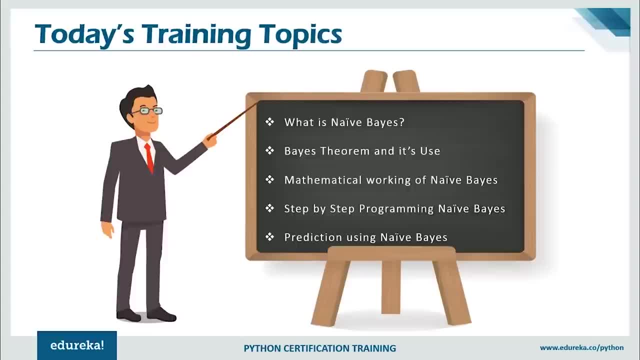 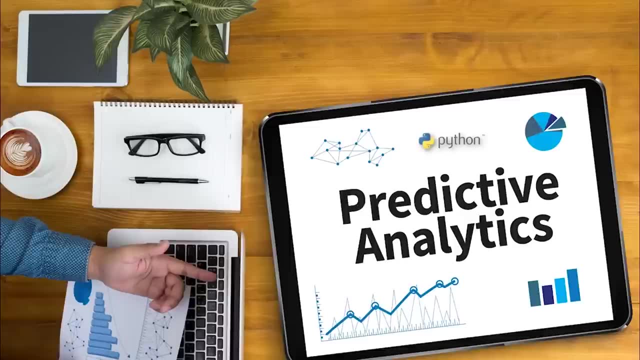 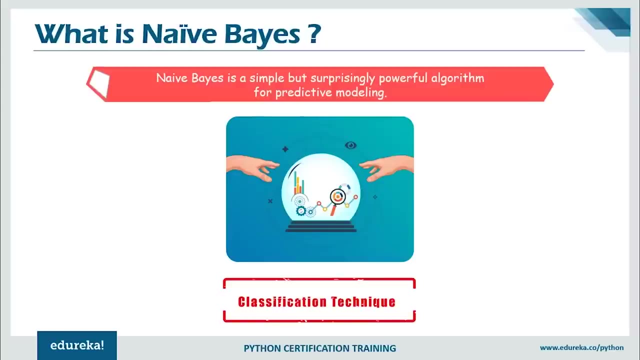 forward. i'll explain the steps involved in the naive bias algorithm one by one and finally, i'll finish off this video with a demo on the naive bias. this is a simple but surprisingly powerful algorithm from predictive analysis. it is a classification technique based on bayes theorem with an assumption of independence among 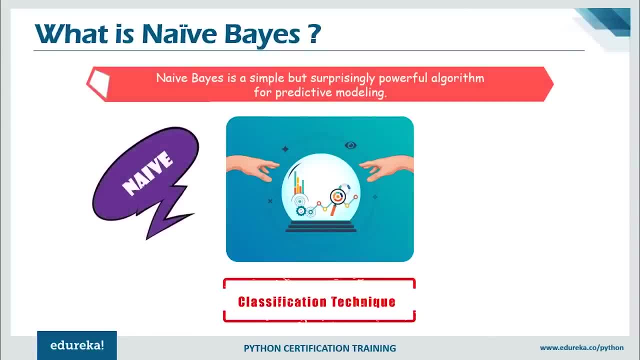 predictors. it comprises of two parts, which is naive and bias. in simple terms, naive bias classifier assumes that the presence of a particular feature in a class is unrelated to the presence of any other feature. even if these features depend on each other or upon the existence of a particular feature in a class, the presence of any other feature is unrelated to the. 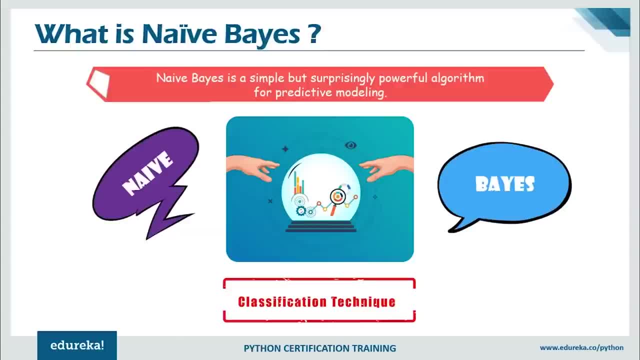 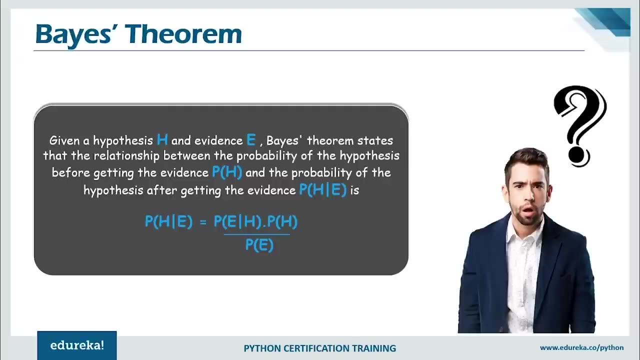 of the other features. all of these properties independently contribute to the probability whether a fruit is an apple or an orange or a banana. So that is why it is known as naive. now, naive based model is easy to build and particularly useful for very last data sets in probability theory and statistics based theorem. 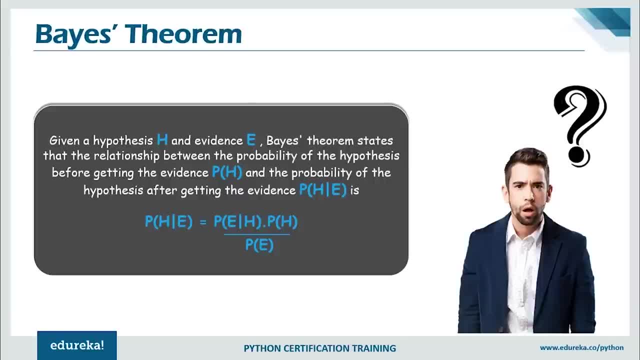 which is already known as the Bayes law or the Bayes rule, describes the probability of an event based on prior knowledge of the conditions that might be related to the event. Now, Bayes theorem is a way to figure out conditional probability. The conditional probability is the probability of an event. 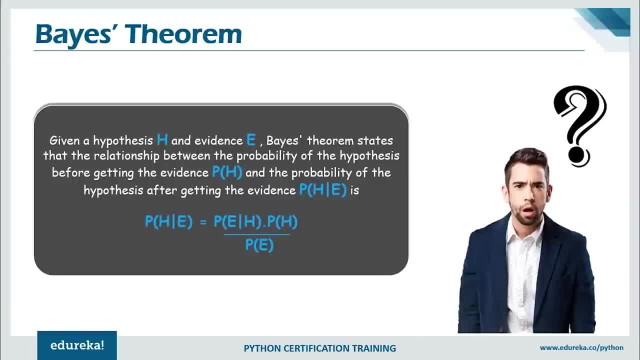 happening, given that it has some relationship to one or more other events. For example, your probability of getting a parking space is connected to the time of the day you park, where you park and what conventions are you going on at. that time based theorem is slightly more nuanced in a nutshell: 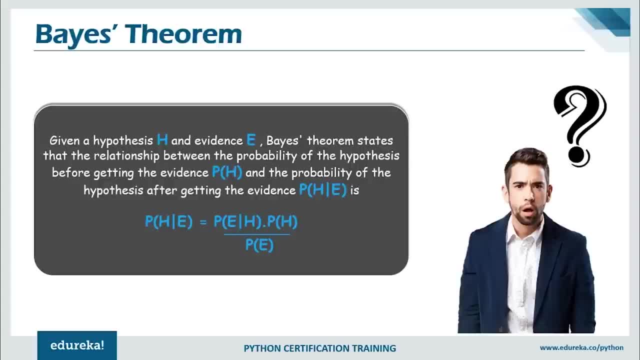 connected to the time of the day you Park, where you Park and what conventions are you going on at that time. based theorem is slightly more nuanced. in a nutshell, It gives you an actual probability of an event given information about the tests. Now, if you look at the definition of Bayes theorem, we can see: 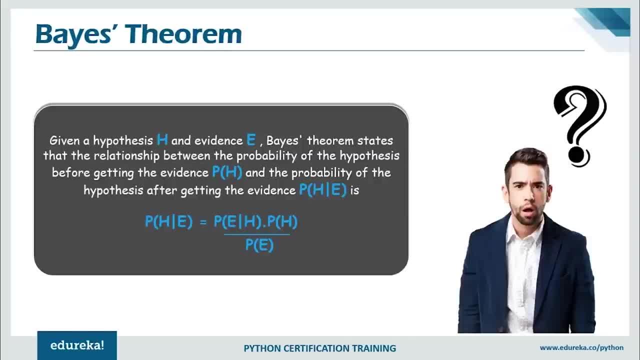 that, given a hypothesis H and the evidence E, Bayes theorem states that the relationship between the probability of the hypothesis before getting the evidence, which is the P of H, and the probability of the hypothesis after getting the evidence, that is, P of H given E, is defined as probability of E given H into probability of H. 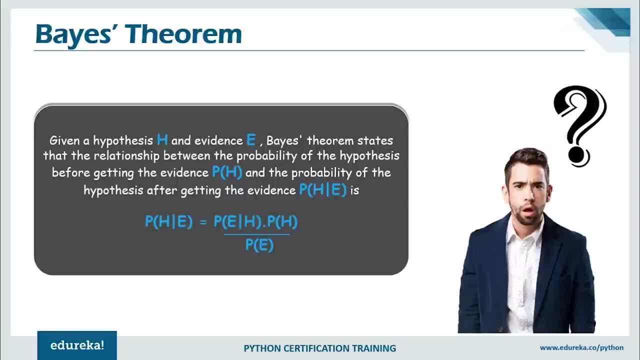 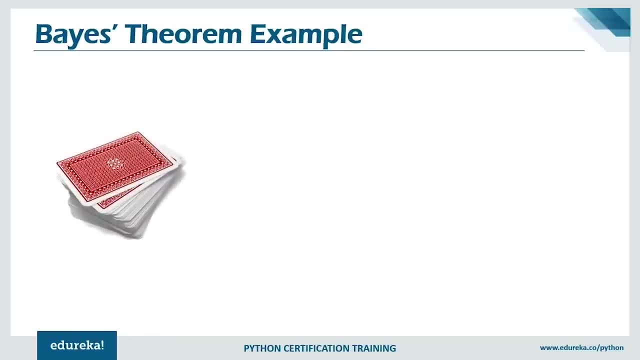 divided by probability of E. It's rather confusing, right? So let's take an example to understand this theorem. So suppose I have a deck of cards and if a single card is drawn from the deck of playing cards, the probability that the 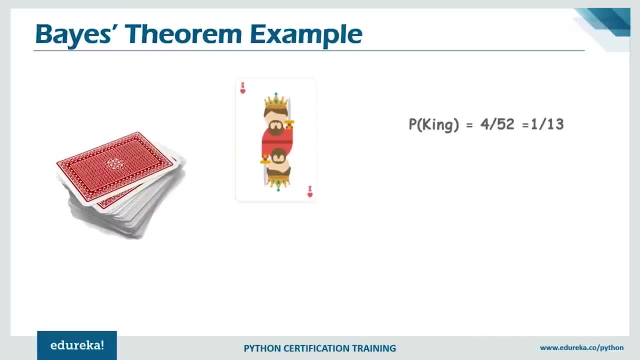 card is a king is 4 by 52, since there are four Kings in a standard deck of 52 cards. Now if King is an event, this card is a king. The probability of King is given as 4 by 52. that is equal to 1. 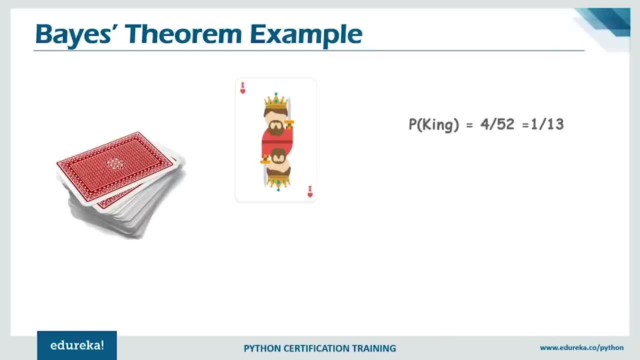 by 13.. Now if the evidence is provided- for instance, someone looks at the card- That the single card is a face card, The probability of King, given that it's a face, can be calculated using the Bayes theorem by this formula: 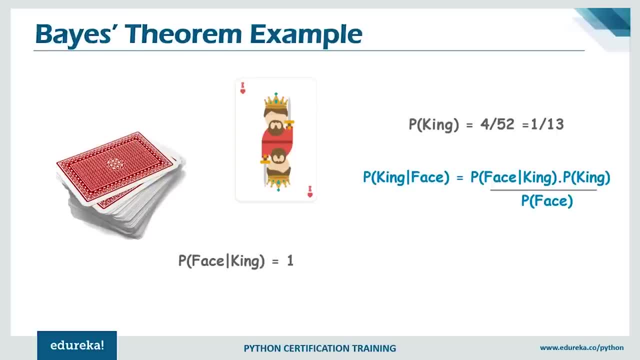 Now, since every King is also a face card, the probability of face, given that it's a king, is equal to 1, and since there are three face cards in each suit, that is, the Jack, King and Queen, the probability of the face card is equal to 12 by 52, that is, 3 by 30. now, using 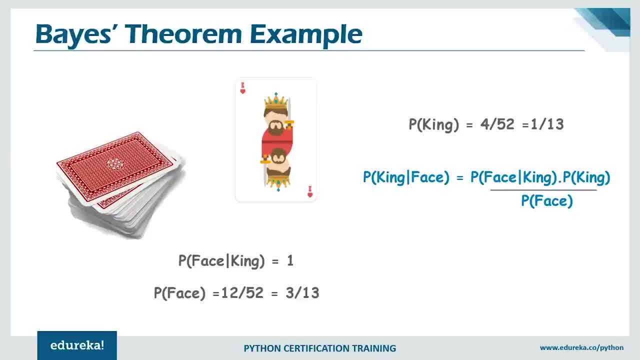 Bayes theorem, We can find out the probability Of King, given that it's a face. So our final answer comes to 1 by 3, which is also true. So if you have a deck of cards which has having only faces, now, 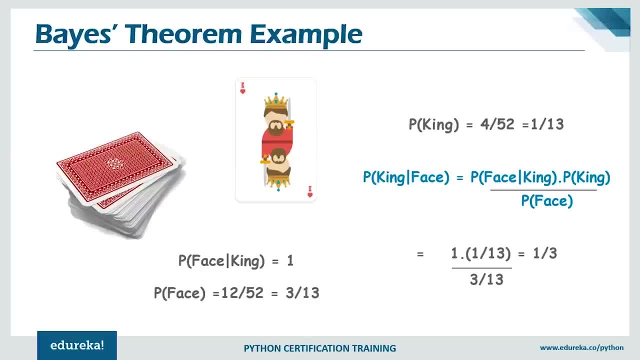 there are three types of phases, which are the Jack, King and Queen. So the probability that it's a king is 1 by 3.. Now, this is the simple example of how Bayes theorem works. Now, if we look at the proof as in how this Bayes theorem evolved, 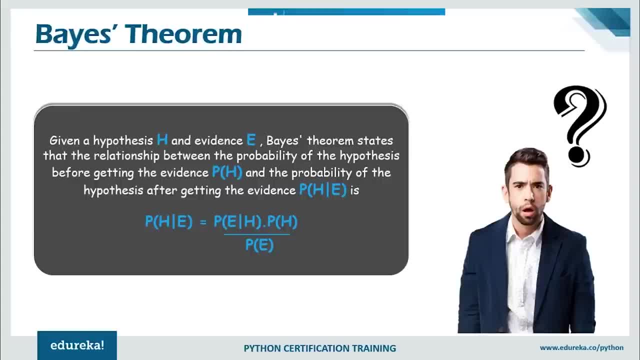 It gives you an actual probability of an event, given information about the tests. Now, if you look at the definition of Bayes theorem, we can see that, given a hypothesis H and the evidence E, Bayes theorem states that the relationship between the probability of the hypothesis before getting the evidence, which is the 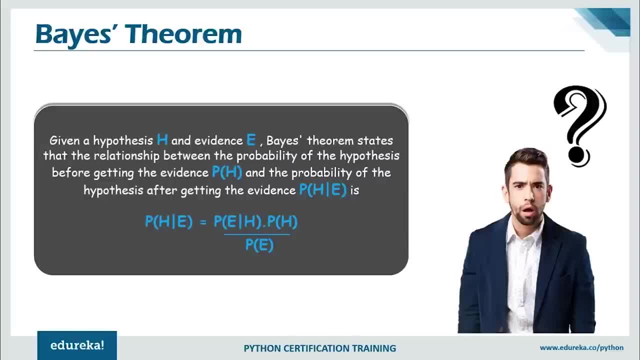 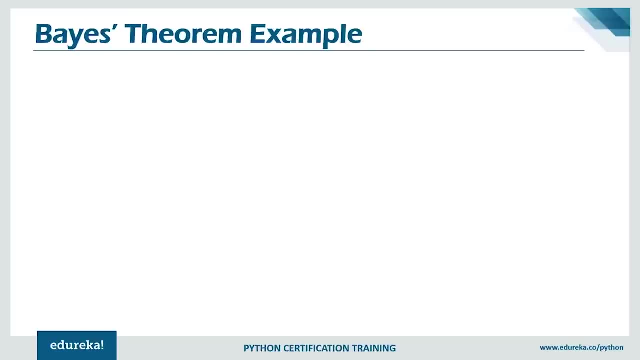 P of H and the probability of the hypothesis after getting the evidence, that is, P of H given E is defined as probability of E given H into probability of H divided by probability of E. it's rather confusing, right? So let's take an example to understand. 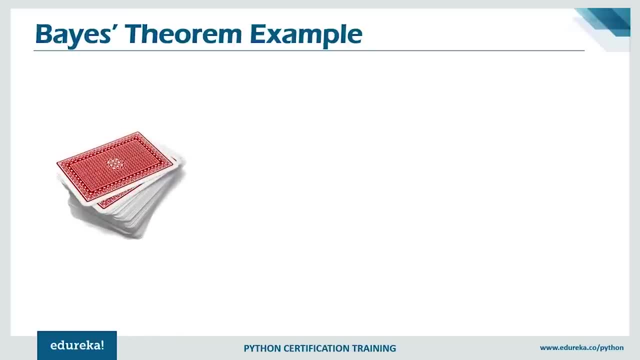 This theorem. So suppose I have a deck of cards and if a single card is drawn from the deck of playing cards, the probability that the card is a king is 4 by 52, since there are four Kings in a standard deck of 52 cards. 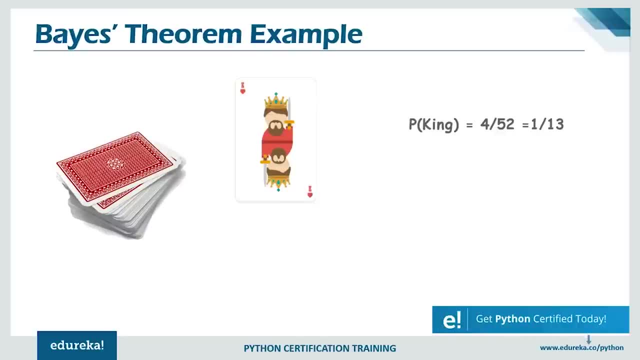 Now if King is an event, this card is a king. The probability of King is given as 4 by 52, that is equal to 1 by 13.. Now if the evidence is provided- for instance someone looks at the card- that the single card is a face card. 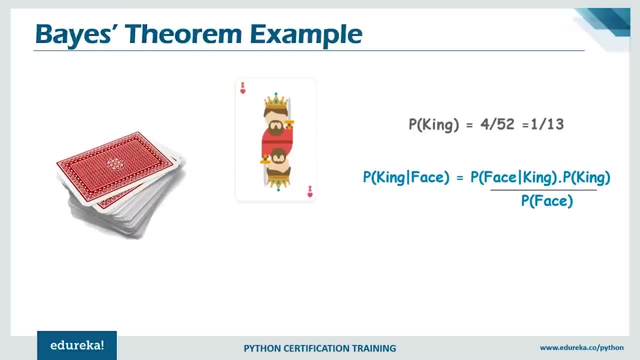 The probability of King, given that it's a face, can be calculated using the Bayes theorem by this formula. Now, since every King is also a face card, the probability of face, given that it's a king, is equal to 1, and since there are three face cards in each suit, that is, the Jack King and 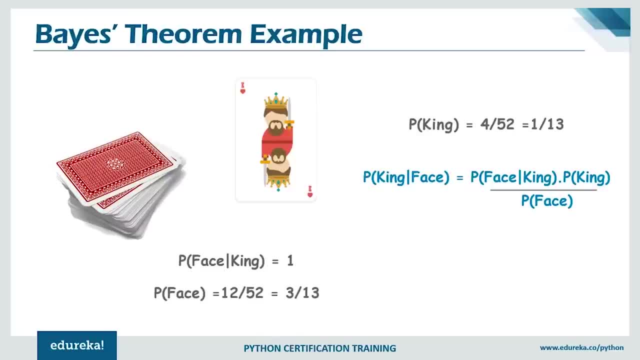 Queen. the probability of the face card is equal to 12 by 52, that is, 3 by 30. Now, using Bayes theorem, we can find out the probability of King, given that it's a face. So our final answer comes to 1 by 3, which is also true. 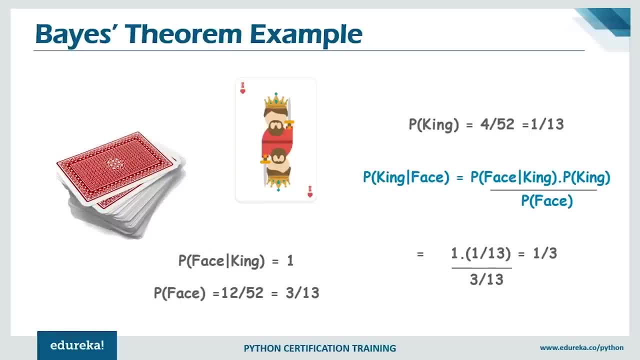 So, if you have a deck of cards which has having only faces, now there are three types of phases which are the Jack, King and Queen. So the probability that it's a king is 1 by 3.. Now this is the simple example of how Bayes theorem works. 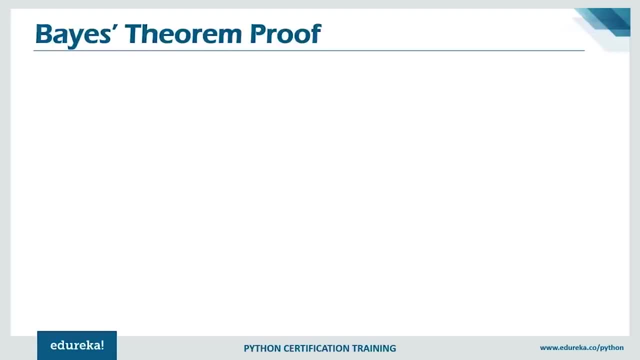 Now if we look at the proof, as in how this Bayes theorem evolved. So here we have probability of A given B And probability of B given A. now for a joint probability distribution over the sets A and B, the probability of A intersection B, the conditional probability of A given B, is: 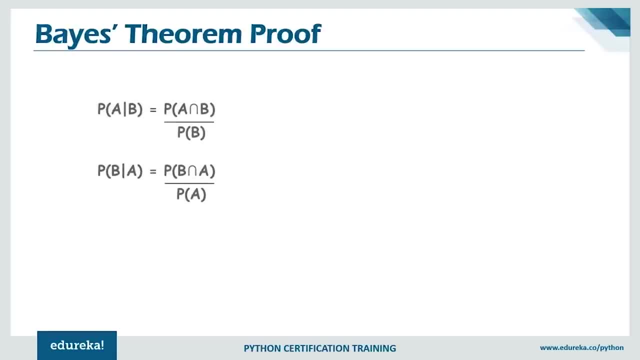 So here we have probability Of a given B and probability of B given a. now for a joint probability distribution over the sets a and B. the probability of a intersection B- the conditional probability of a given B, is defined as the probability of a intersection B divided by probability of B, and similarly. 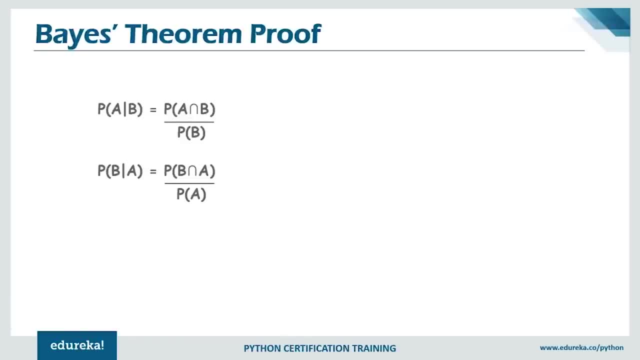 probability of B given a is defined as probability of B intersection a divided by probability of a. now we can equate probability of a intersection B and probability Of B intersection a, as both are the same thing. now, from this method, as you can see, we get our final Bayes theorem proof, which is the: 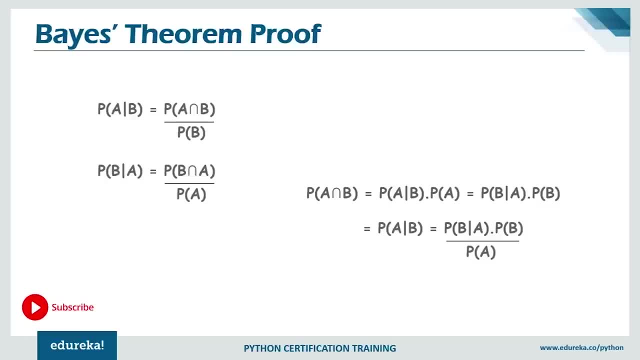 probability of a given B equals probability of B given a into probability of B divided by the probability of a. now, while this is the equation that applies to any probability distribution over the events a and B, it has a particular nice interpretation in case where a is represented as the hypothesis, H and B is represented as some. 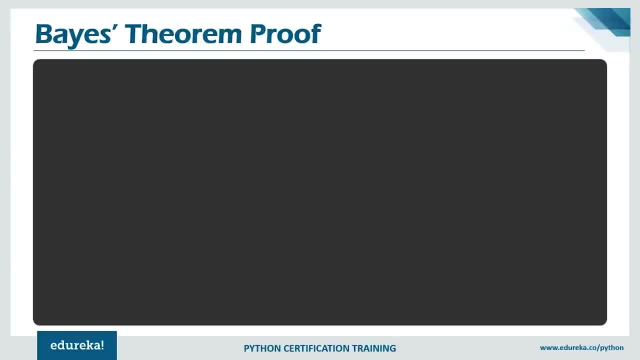 of Observed evidence E. in that case the formula is: P of H given E is equal to P of E given H into probability of H divided by probability of E. now this relates the probability of hypothesis before getting the evidence, which is P of H, to the probability of the hypothesis. 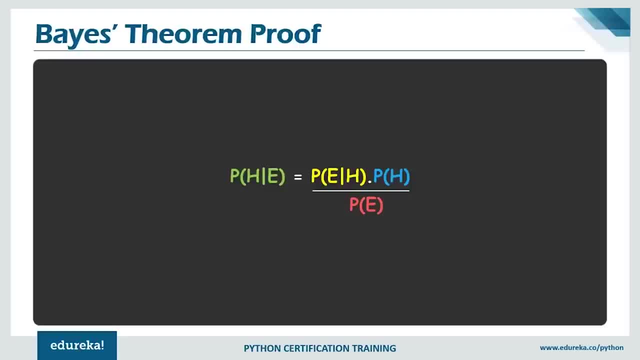 after getting the evidence, which is P of H given E. for this reason, P of H is known as the prior probability, while P of H given E is known as the posterior probability, And the factor that relates the two is known as the likelihood ratio. now, using these terms, Bayes theorem can be rephrased as the: 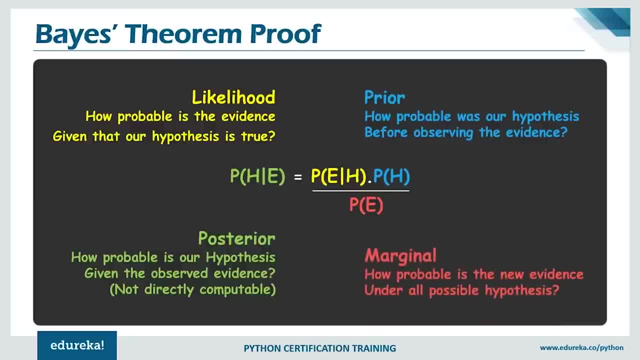 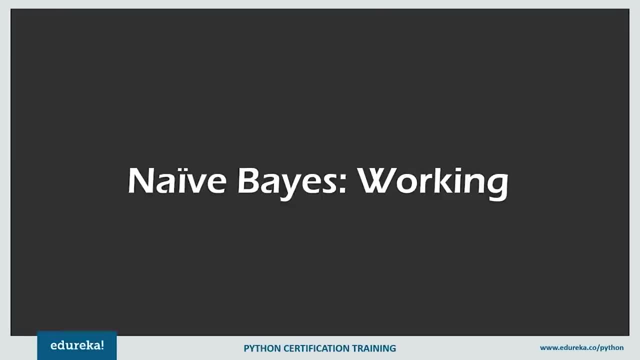 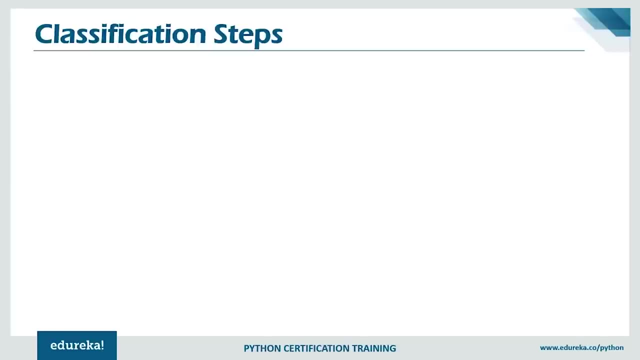 procedure. probability equals the prior probability times the likelihood ratio. So now that we know the math which is involved behind the Bayes theorem, let's see how we can implement this in a real-life scenario. So suppose we have a data set in which we have the outlook, the human 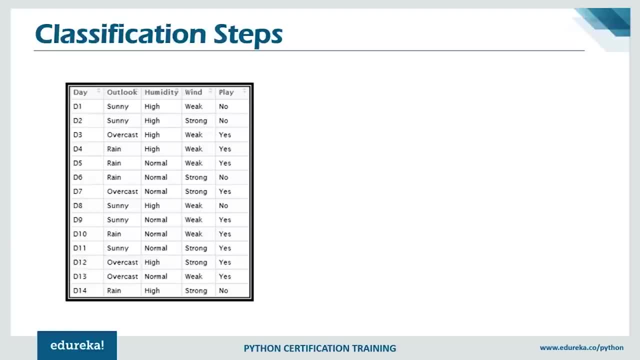 entity and we need to find out whether we should play or not on that day. So the outlook can be sunny, overcast, rain and the humidity are high, normal, and the wind are categorized into two features, which are the weak and the strong winds. the first of all will 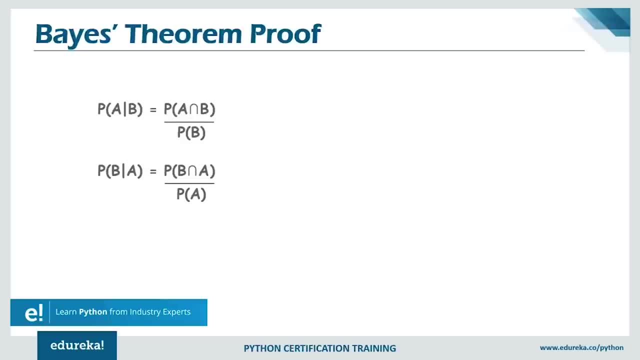 defined as the probability of A intersection B divided by probability of B, and similarly, probability of B given A is defined as probability of B intersection A divided by probability of A. now we can equate probability of A intersection B and probability of B intersection A as both. 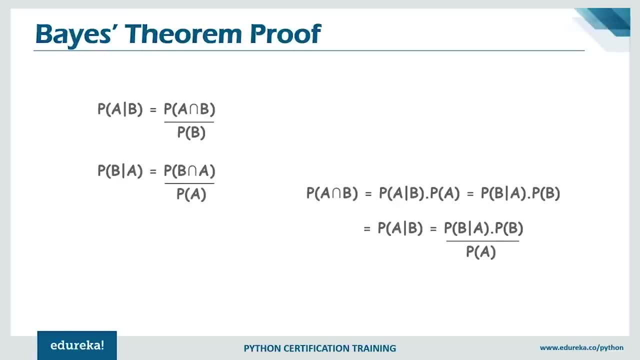 are the same thing. Now, from this method, as you can see, we get our final base theorem proof, which is: the probability of A given B equals probability of B given A into probability of B divided by the probability of A. Now, while this is the equation that applies to any probability distribution over, 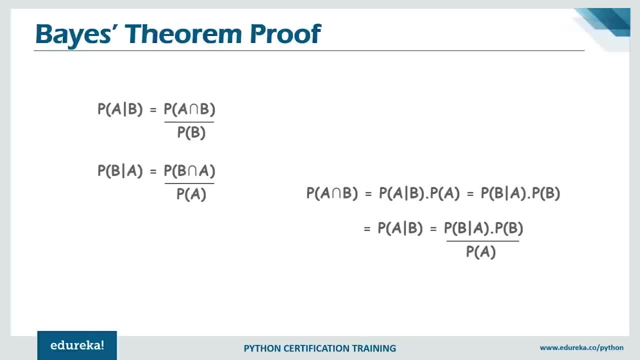 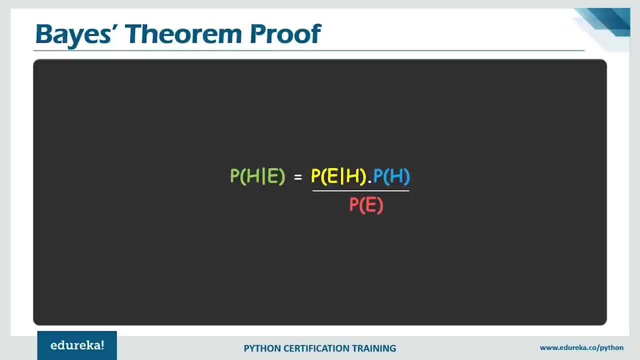 the events A and B. it has a particularly nice interpretation in case where A is represented as the hypothesis H and B is represented, as some observed evidence, E. In that case the formula is: P of H given E is equal to P of E given H into probability of H divided by probability of E. 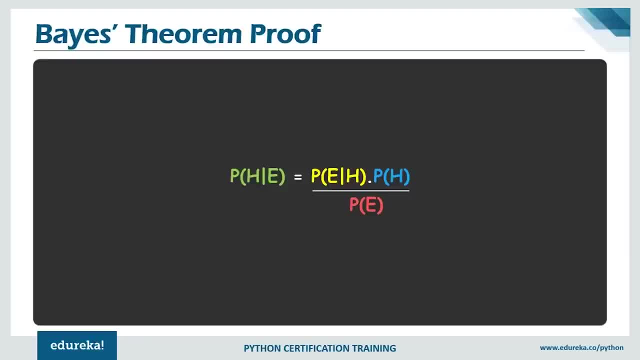 Now this relates the probability of hypothesis before getting the evidence, which is P of H, to the probability of the hypothesis after getting the evidence, which is P of H given E. For this reason, P of H is known as the prior probability, While P of H given E is known as the posterior probability and the factor that relates the two. 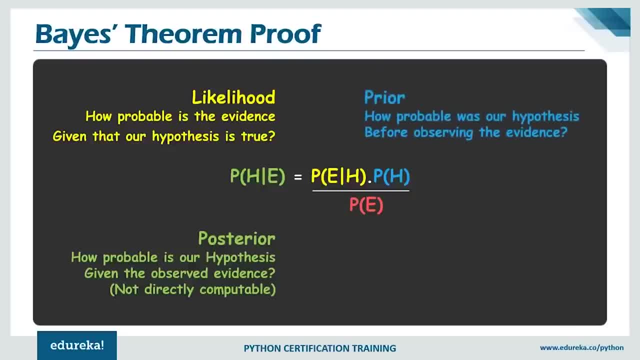 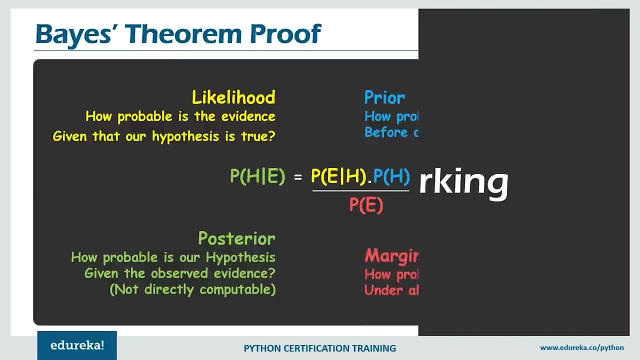 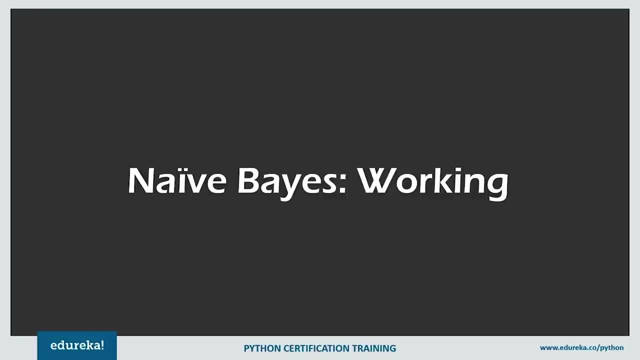 is known as the likelihood ratio. Now, using these terms, base theorem can be rephrased as: the posterior probability equals the prior probability times the likelihood ratio. So now that we know the maths which is involved behind the base theorem, let's see how we can implement this in a real life scenario. 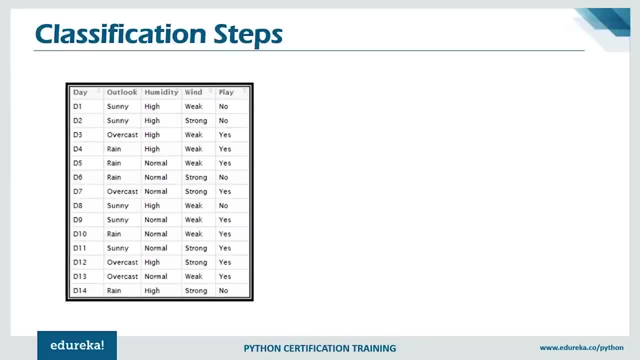 So suppose we have a data set in which we have the outlook, the humidity, and we need to find out whether we should play or not on that day. So the outlook can be sunny, overcast, rain and the humidity are high, normal, and the wind are categorized into two features which are the weak. 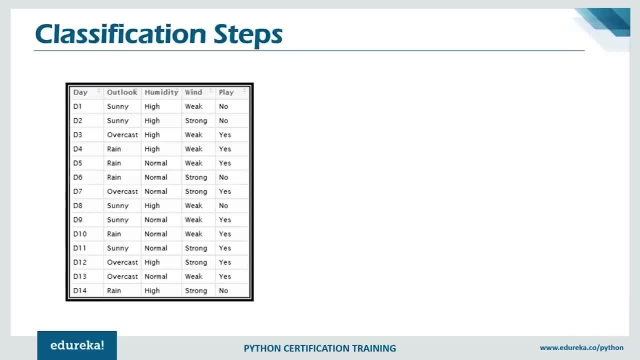 and the strong winds. Now, first of all, we'll create a frequency table using each attribute of the data set. So the frequency table for the outlook looks like this: we have sunny, overcast and rainy. the frequency table of humidity and the humidity are high, normal and the wind are categorized into two. 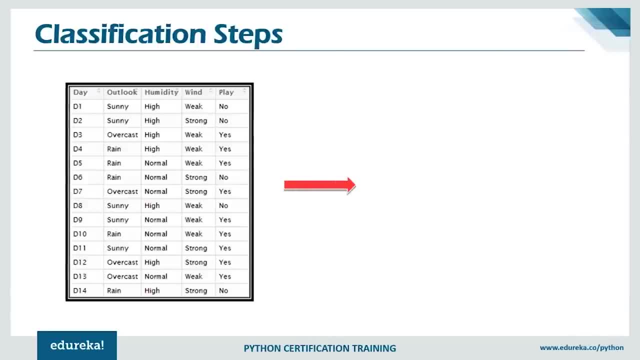 create a frequency table using each attribute of the data set. So the frequency table for the outlook looks like this: We have sunny, overcast and rainy. the frequency table of humidity looks like this and the frequency table of wind looks like this: We have strong and weak for wind and high and normal ranges for. 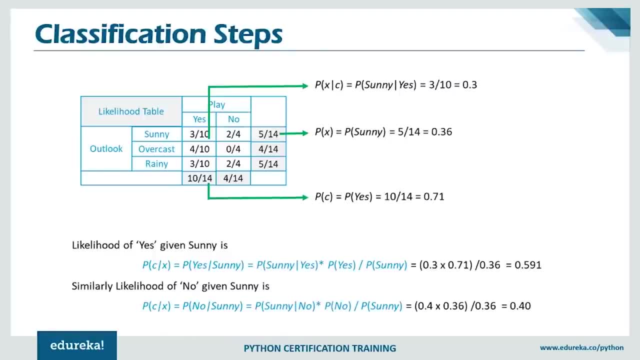 humidity. So for each frequency table, we will generate a likelihood table. now, Now the likelihood table contains the probability of a particular day. Suppose we take the sunny and we take the play as yes and no. So the probability of Sunny, given that we play. 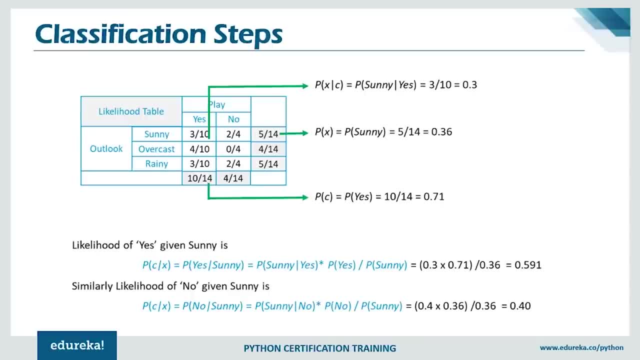 Yes, is 3 by 10, which is 0.3. the probability of X, which is the probability of Sunny, is equal to 5 by 14.. Now, These are all the terms which are just generated from the data which we have here. 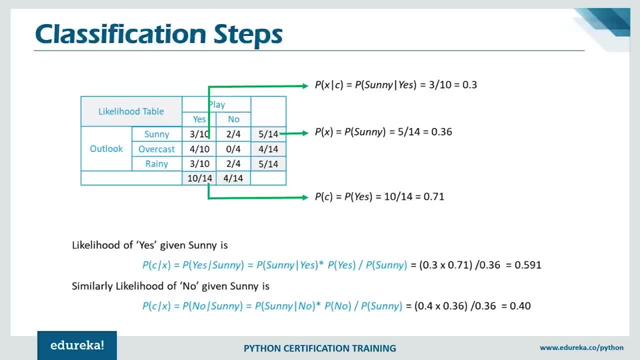 And finally, the probability of yes is 10 out of 14.. So if we have a look at the likelihood of yes, given that it's a sunny, we can see using base theorem It's the probability of Sunny given yes into probability of yes divided by the probability of Sunny. 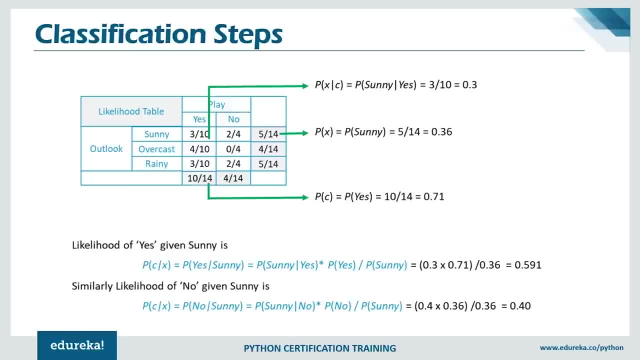 So we have all the values here calculated. So if you put that in our base theorem equation, we get the likelihood of yes as 0.59.. Similarly the likelihood of no can also be calculated here: It's 0.40.. 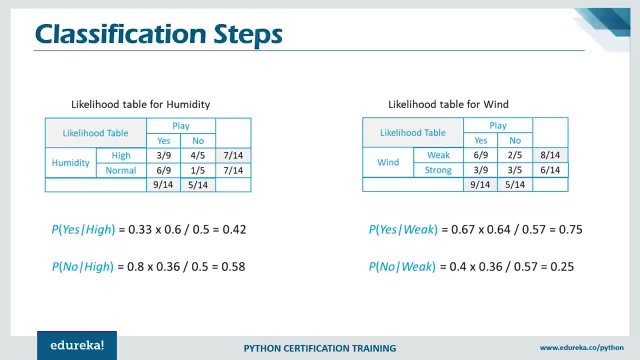 Now, Similarly, we are going to create the likelihood table for both the humidity and the wind. as a. for humidity, The likelihood for yes, given the humidity is high, is equal to 0.42, and the probability of playing no, given the wind is high. 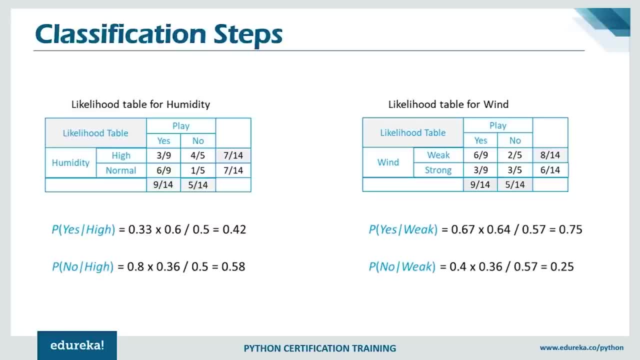 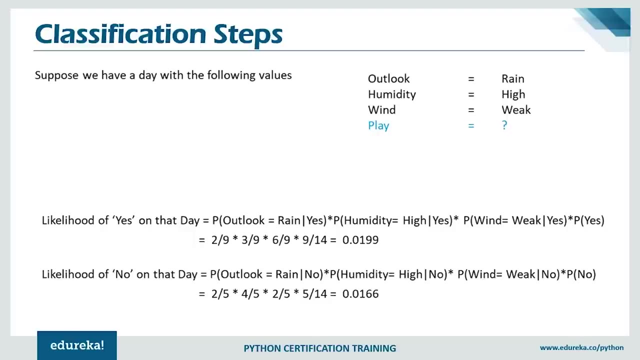 is 0.58.. Now, similarly, for table wind, the probability of yes, given that the wind is weak, is 0.75 and the probability of no, given that the wind is weak, is 0.25.. Now suppose we have a day which has high rain, which has high 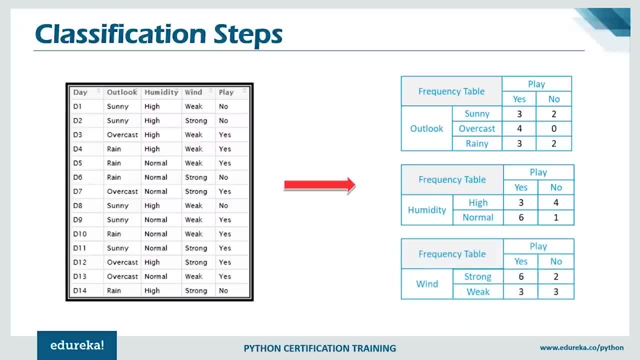 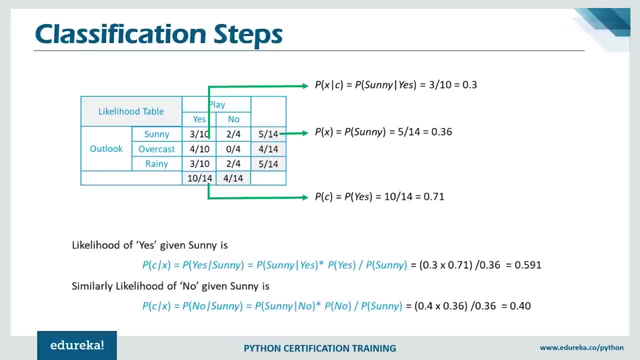 features. So the frequency table of humidity looks like this and the frequency table of wind looks like this. We have strong and weak for wind and high and normal ranges for humidity. So for each frequency table, we will generate a likelihood table now. Now the likelihood table contains: 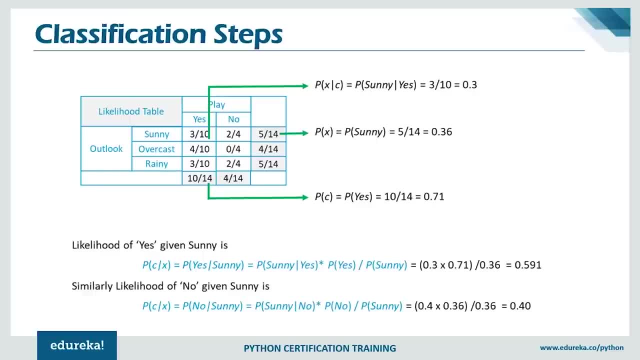 the probability of a particular day. suppose we take the sunny and we take the play as yes and no. so the probability of sunny, given that we play yes, is 3 by 10, which is 0.3.. The probability of x, which is the probability of sunny, is equal to 5 by 14.. Now, these are all the terms, which are just. 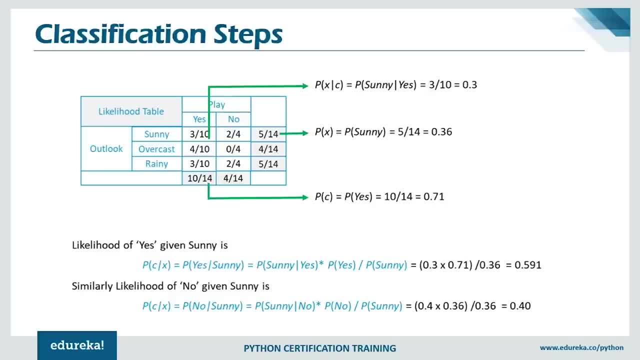 generated from the data which we have here. and finally, the probability of yes is 10 out of 14.. So if we have a look at the likelihood of yes, given that it's a sunny, we can see using base theorem it's the probability of sunny, given yes into probability of yes divided by the probability. 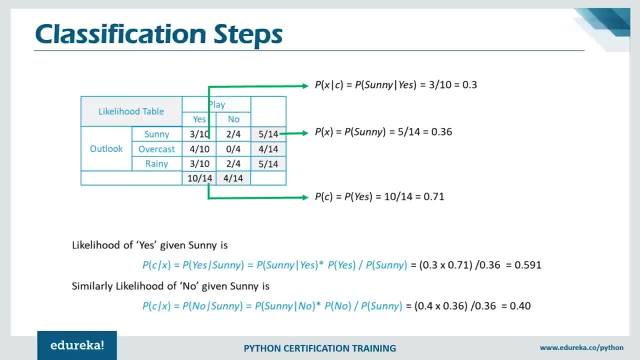 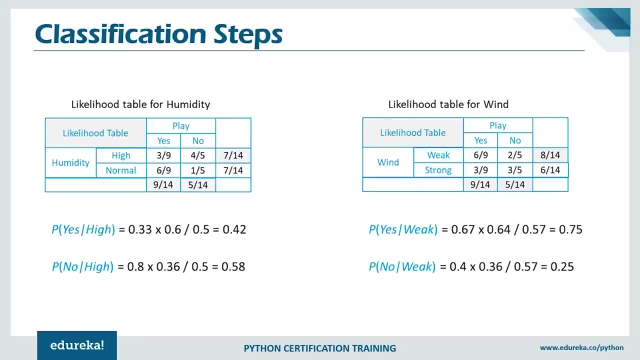 of sunny. So we have all the values here calculated. so if we put that in our base theorem equation, we get the likelihood of yes as 0.59.. Similarly the likelihood of no can also be calculated. here it's 0.40.. Now, similarly, we are going to create the likelihood table for both the humidity and 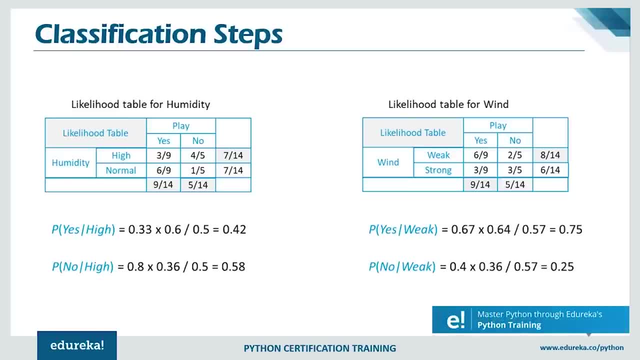 the wind. So, for humidity, the likelihood for yes, given the humidity is high, is equal to 0.42, and the probability of playing no, given the wind is high, is 0.58.. Similarly, for table wind, the probability of yes, given that the wind is weak, is 0.75 and the 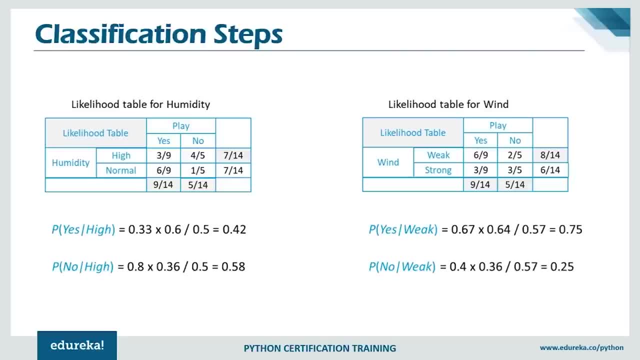 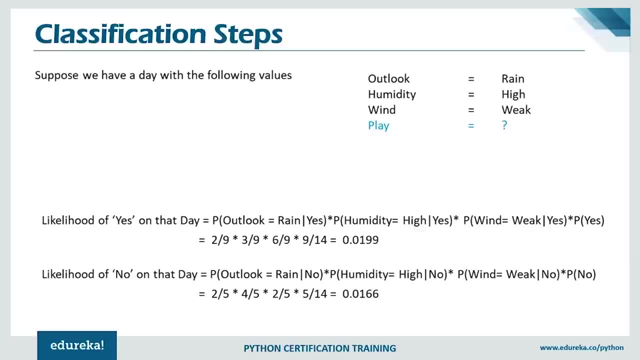 probability of no, given that the wind is weak, is 0.25.. Now suppose we have a day which has high rain, which has high humidity and the wind is weak. So should we play or not Now? so for that we use the base theorem. here again, The likelihood of yes on that day is equal to the probability of. 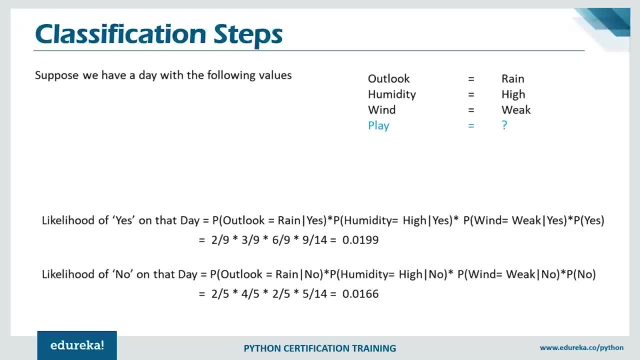 outlook: rain, given the humidity, and the wind is weak. So for that we use the base theorem here, given that it's a yes into probability of humidity, given that it's a yes and the probability of wind that is weak, given that it's, we are playing yes into the probability of yes, which equals to 0.019. 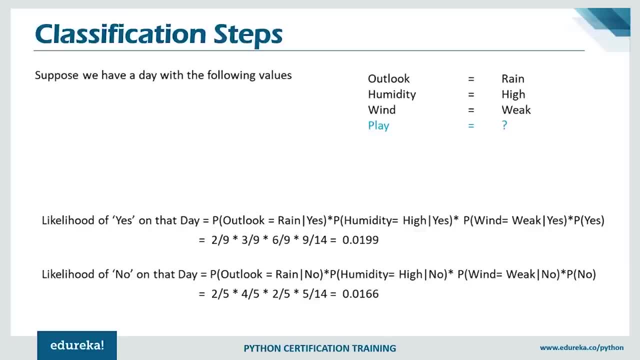 humidity and the wind is weak. So should we play or not Now? so for that we use the base theorem. here again, The likelihood of yes on that day is equal to the probability of outlook rain, given that it's a yes into probability of humidity. 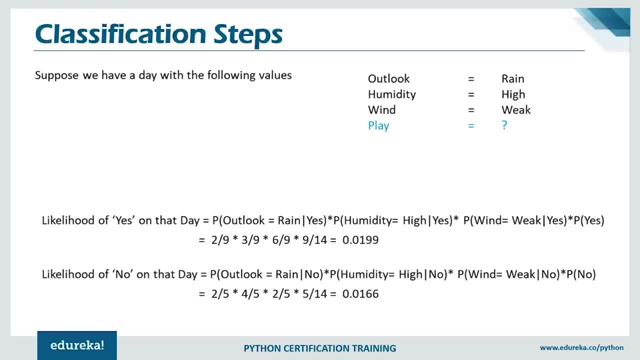 given that it's a yes And the probability of wind that is weak given that it's, we are playing yes into the probability of yes, which equals to 0.019, and similarly, the likelihood of no on that day is equal to 0.016.. 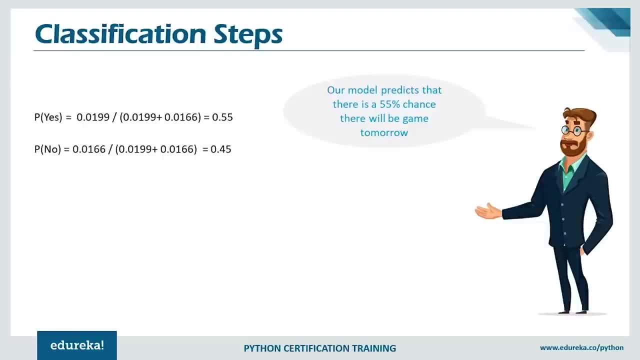 Now, if we look at the probability of yes for that day of playing, we just need to divide it with the likelihood sum of both the yes and no. So the probability of playing tomorrow, which is yes, is 0.5, whereas the probability of Not playing is equal to 0.45.. 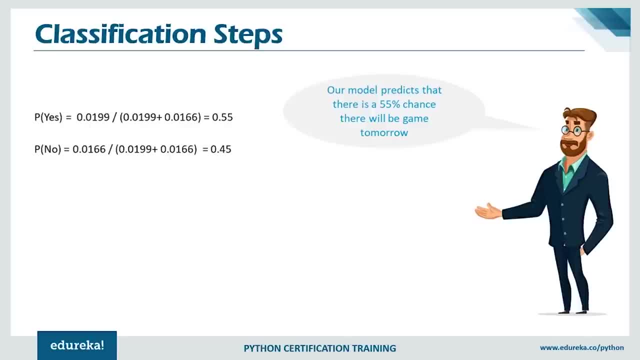 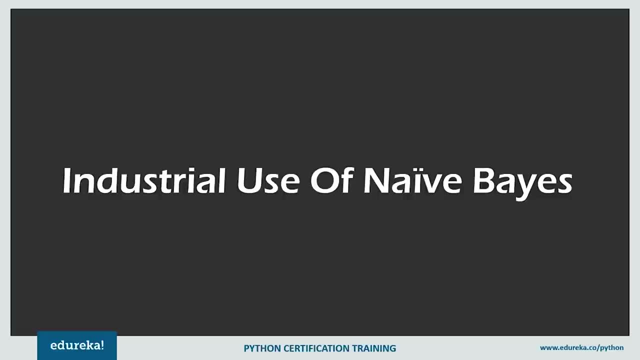 But this is based upon the data which we already have with us. So now that you have an idea of what exactly is naive bias, how it works, and we have seen how it can be implemented on a particular data set, Let's see where it is used in the industry. 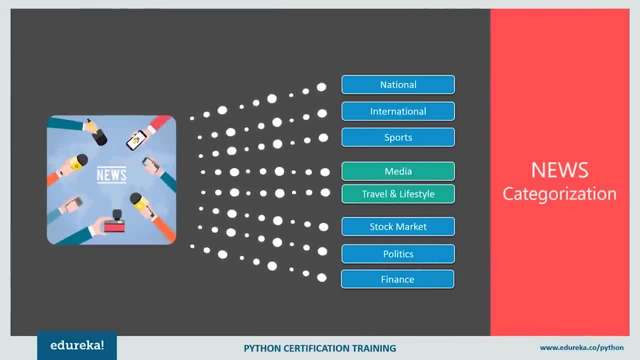 Now starting with our first industrial use case, which is news categorization, or we can use the term text classification To broaden the spectrum of this algorithm. news in the web are rapidly growing in the era of information age, where each new site has its own different layout and categorization for grouping. 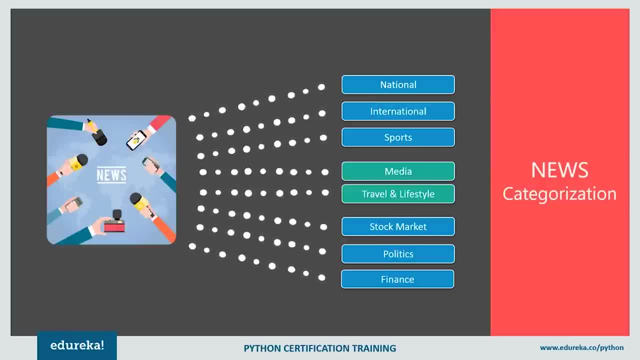 news. Now. these heterogeneity of layout and categorization cannot always satisfy individual users. need to remove these heterogeneity, and classifying the news articles according to the user preference is a formidable task. companies use web crawler to extract useful text from HTML pages- The news articles- and each of these news articles is then tokenized. 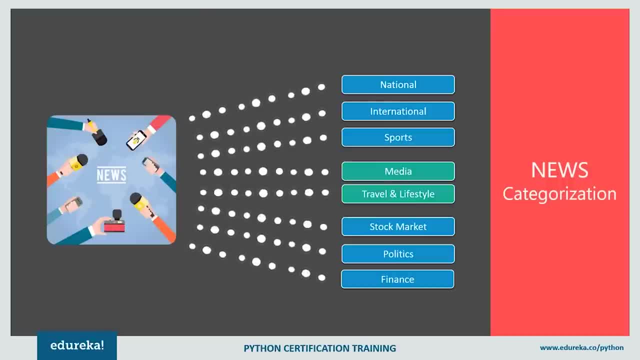 not. these tokens are nothing but the categories of the news. now, in order to achieve better classification result, we remove the less significant words, which are the stop words, from the documents or the articles, and then we apply the naive bias classifier for classifying the news contents based on the news code. 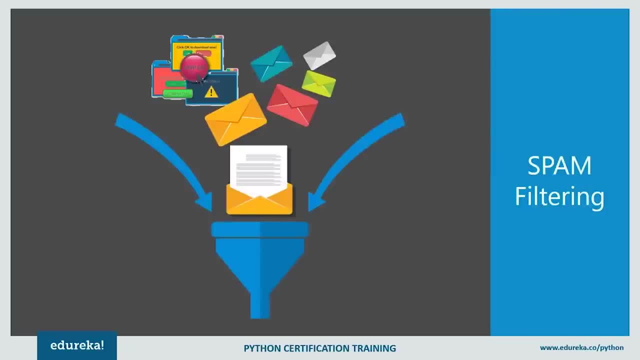 Now this is by far one of the best examples of naive bias classifier, which is spam filtering. Now it's. the naive bias classifier are a popular statistical technique for email filtering. They typically use bag-of-words features to identify the spam email, an approach commonly used in text classification as well. 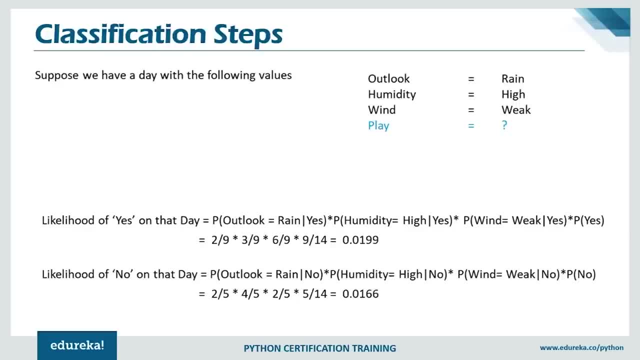 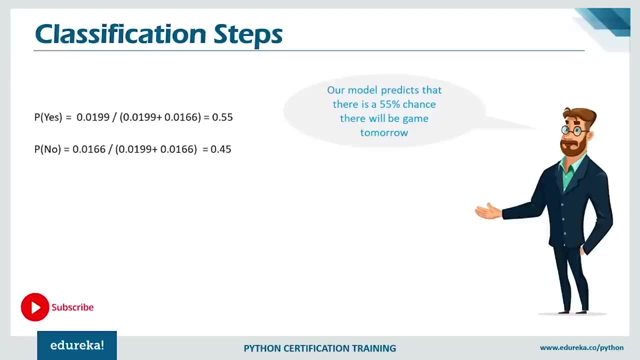 and similarly, the likelihood of no on that day is equal to 0.016.. Now, if we look at the probability of yes for that day of playing, we just need to divide it with the likelihood sum of both the yes and no. So the probability of playing no is equal to 0.019 and the probability of playing no is equal to 0.016. 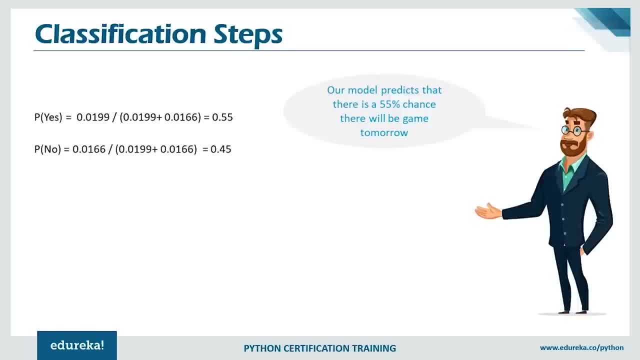 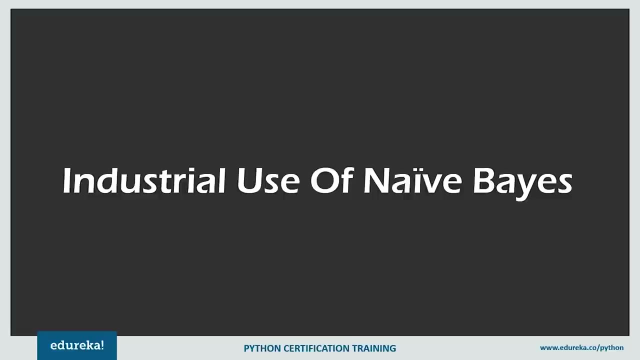 So the probability of playing tomorrow, which is yes, is 0.5, whereas the probability of not playing is equal to 0.45.. Now, this is based upon the data which we already have with us. So now that you have an idea of what exactly is naive bias, how it works. 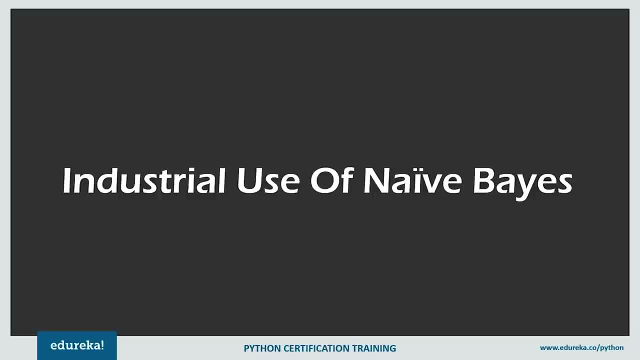 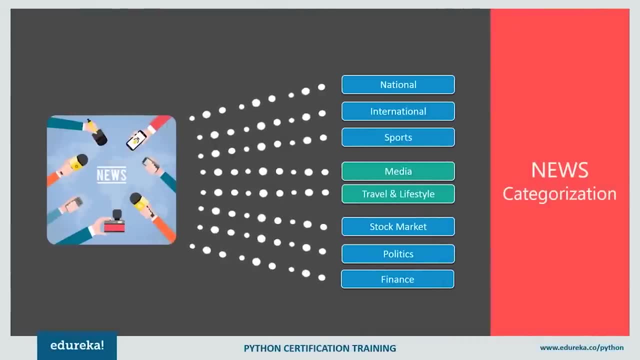 and we have seen how it can be implemented on a particular data set. Let's see where it is used in the industry Now, starting with our first industrial use case, which is categorization, or we can use the term text classification to broaden the spectrum of this. 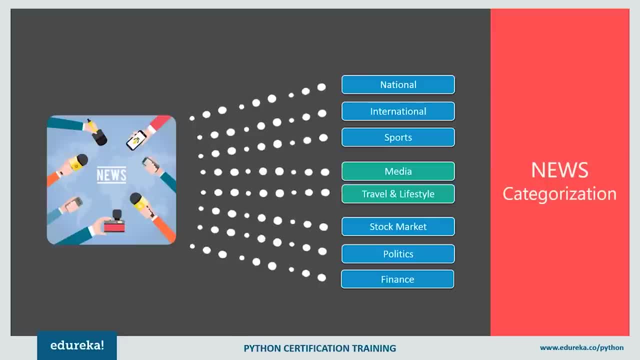 algorithm. news in the web are rapidly growing in the era of information age, where each new site has its own different layout and categorization for grouping news. Now these heterogeneity of layout and categorization cannot always satisfy individual users need to remove these heterogeneity, and classifying the news articles according to the user preference is a formidable task. 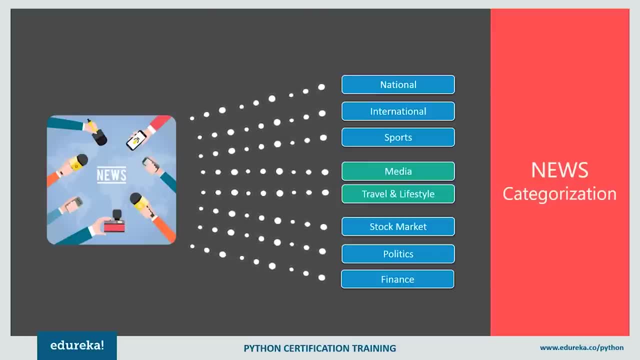 Companies use web crawler to extract useful text from HTML pages- the news articles- and each of these news articles is then tokenized. Now, these tokens are nothing but the categories of the news. now, in order to achieve better classification result, we remove the less significant words, which are the stop words, from the documents or the articles, and then we apply the naive bias. 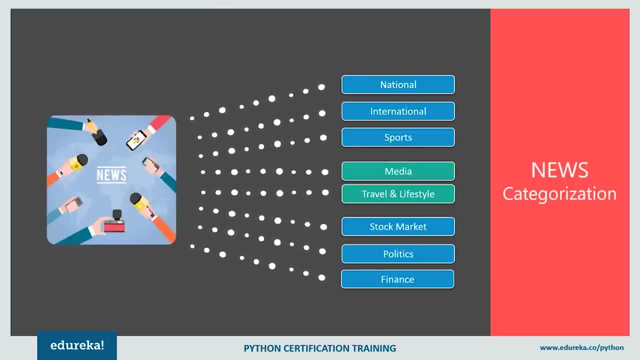 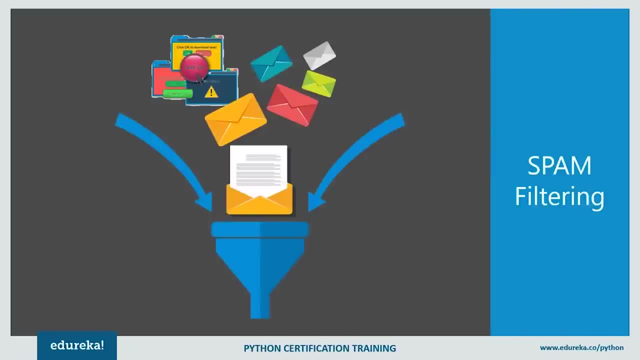 classifier for classifying the news contents based on the news code. Now, this is by far one of the best examples of naive bias classifier, which is spam filtering. Now it's the naive bias classifier are a popular statistical technique for email filtering. They typically use bag of words features. 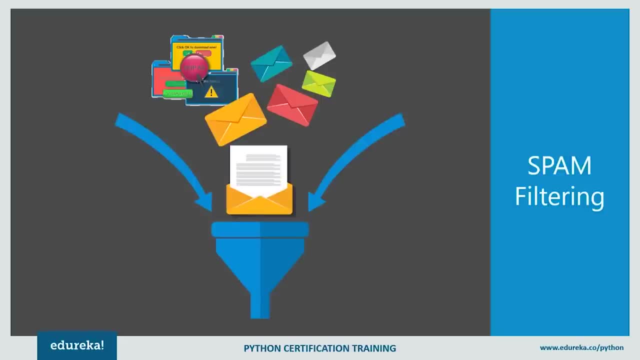 to identify the spam email, an approach commonly used in text classification as well. Now it works by correlating the use of tokens but the spam and the non-spam emails, and then the base theorem, which I explained earlier, is used to calculate the number of words that are used to identify the. 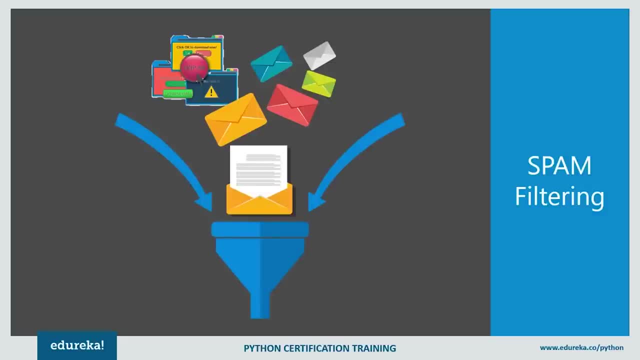 Now it works by correlating the use of tokens but the spam and the non-spam emails, and then the base theorem which I explained earlier is used to calculate the probability that an email is spam or not a spam. So naive bias spam filtering is a baseline technique for dealing. 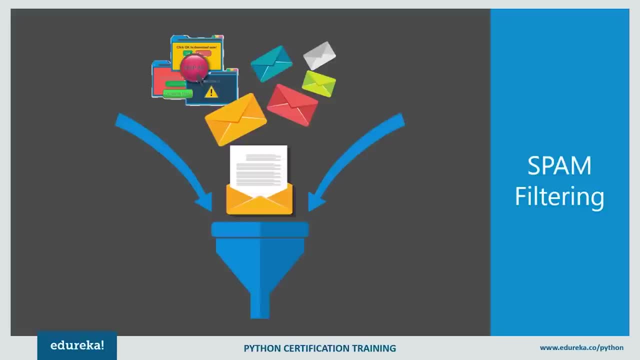 with spam that can tailor itself to the emails need of an individual user and give low-force, positive spam detection rates that are generally acceptable to users. It is one of the oldest ways of doing spam filtering, with its roots in the 1990s. particular words have particular probabilities. 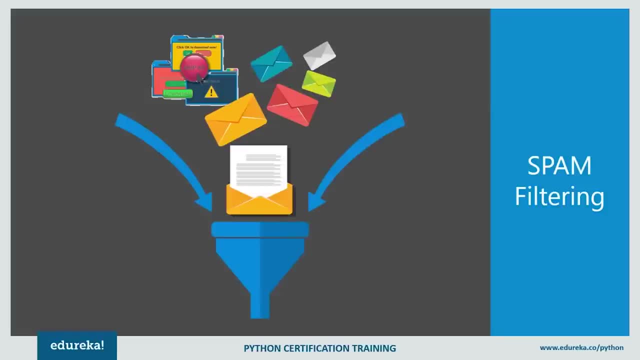 of occurring in spam email and in legitimate email as well. For instance, most emails users will frequently encounter the word lottery or the lucky draw is spam email, but will seldom see it in other emails. The filter doesn't know these probabilities in advance and must. 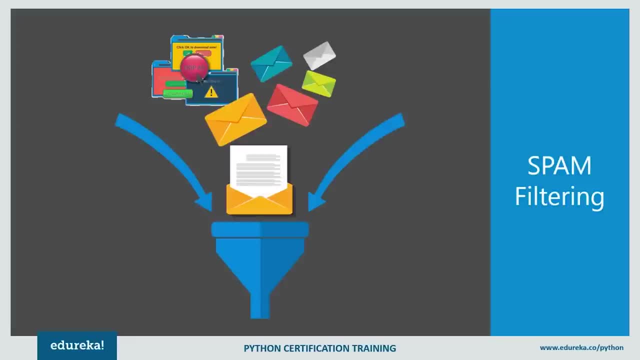 be trained so it can build them up. to train the filter, The user must manually indicate whether a new email is spam or not. for all the words in each training email. The filter will adjust the probability that each word will appear in a spam or legitimate email in the database. 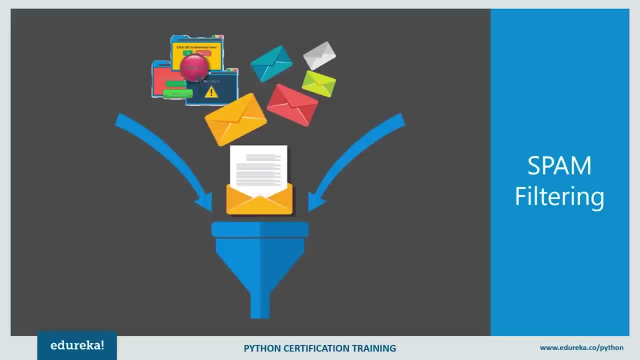 Now, after training the word probabilities, also known as the likelihood functions, I used to compute the probability that an email with a particular set of words, as it belongs to either category, each word in the email contributes the email spam property. This contribution is called the posterior probability and is 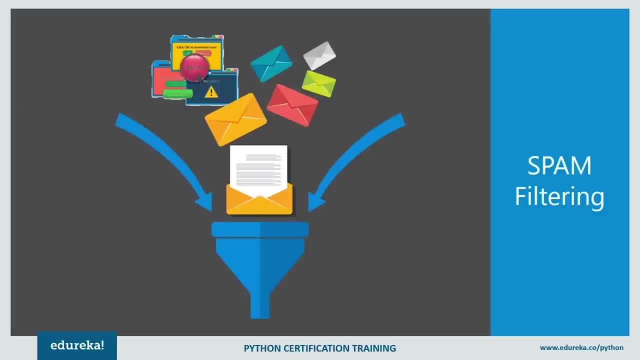 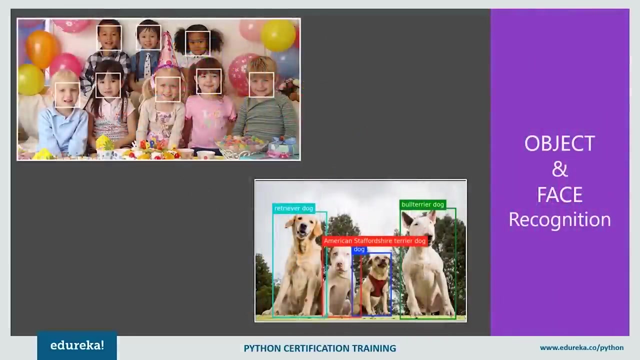 computed again using the base theorem. Then the email spam probability is computed over all the words in the email and if the total exceeds a certain threshold, say 90 or 95%, the filter will mark the email as spam. now, object detection Is the process of finding instances of real-world objects such 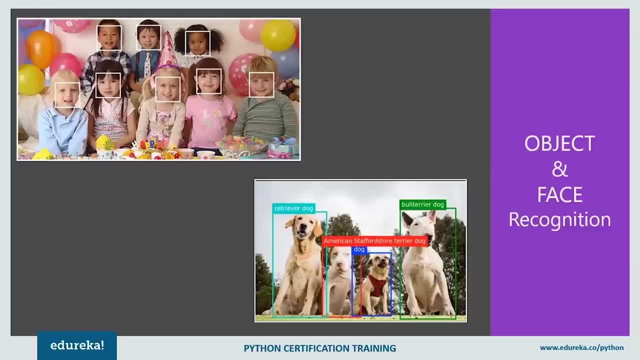 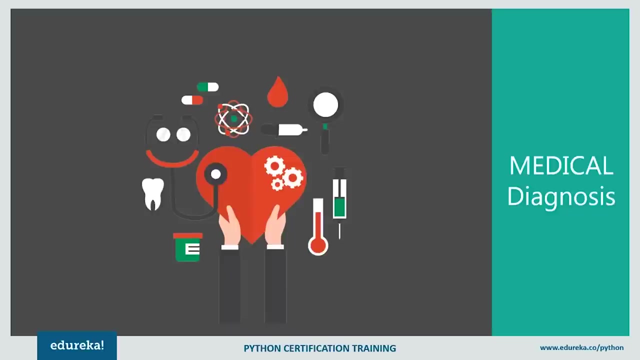 as faces, bicycles and buildings in images of video. now, object detection algorithm typically use extracted features and learning algorithm to recognize instance of an object category. here again, nearby's plays an important role of categorization and classification of object. now, medical area produces increasingly voluminous amount of electronic data, which are becoming more and more complicated. 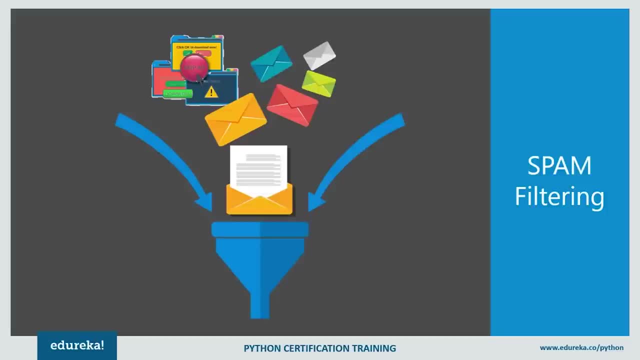 spam email and to calculate the probability that an email is or not a spam. So naive bias. spam filtering is a baseline technique for dealing with spam that can tailor itself to the email's need of an individual user and give low force positive spam detection rates that are generally acceptable to. 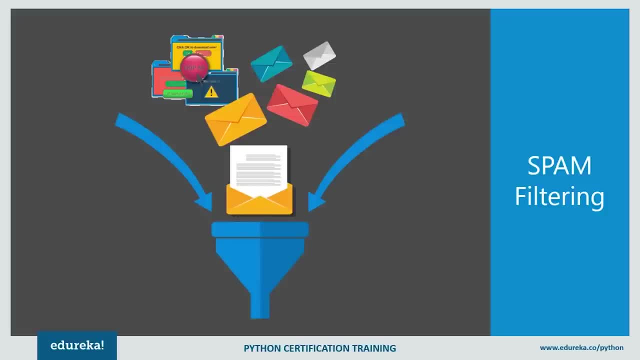 users. It is one of the oldest ways of doing spam filtering, with its roots in the 1990s. Particular words have particular probabilities of occurring in spam email and in legitimate email as well. For instance, if you have a spam email and you have a spam email and you have a spam email and you 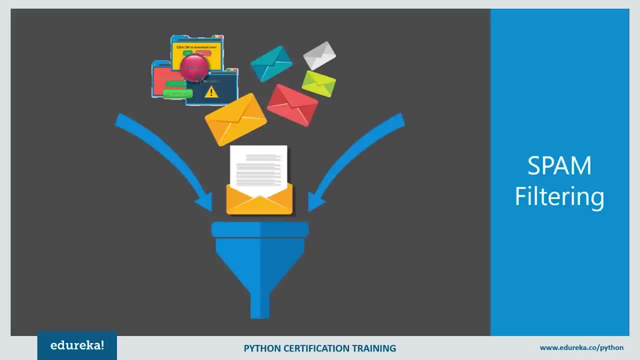 have spam spam filter to identify whether you know a spam email or not, and you have transparency data. that also Sure. you can alsoчеop the spam email as a form of egg trading. This will as well enable you to manually sentir all of your spam emails, and 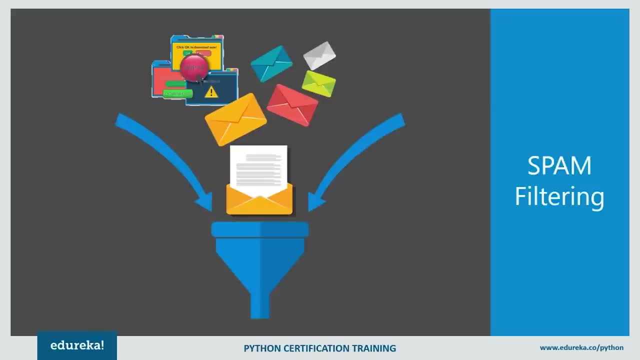 able to start using some policies that centered around that automated smelter to steal snot. probabilities, also known as the likelihood functions, are used to compute the probability that an email with a particular set of words as it belongs to either category. each word in the email contributes the email spam probability. 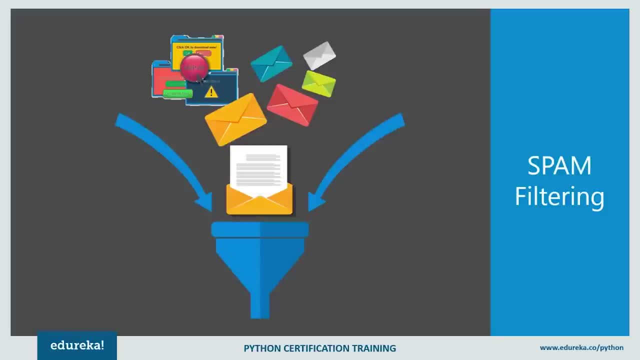 this contribution is called the posterior probability and is computed again using the Bayes theorem. then the email spam probability is computed over all the words in the email and if the total exceeds a certain threshold, say 90 or 95 percent, the filter will mark the email as spam. now, object detection is: 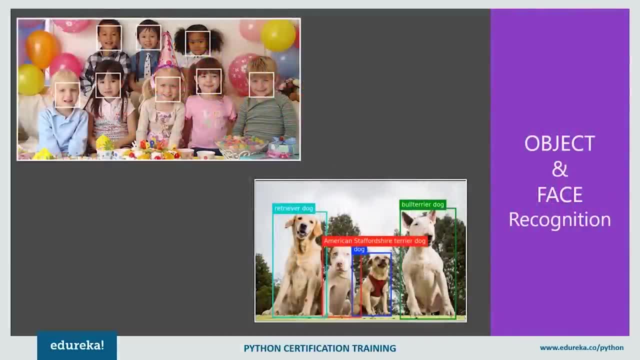 the process of finding instances of real-world objects such as faces, bicycles and buildings in images of video. now, object detection algorithm typically use abstracted features and learning algorithm to recognize instance of an object category. here again, name buys plays an important role of categorization and classification of object. now, medical area produces. 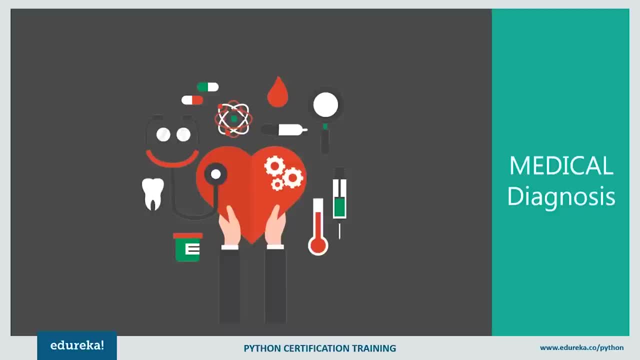 increasingly voluminous amount of electronic data, which are becoming more and more complicated. the produced medical data have certain characteristics that make their analysis very challenging and attractive as well. among all the different approaches, the naive bias is used. it is the most effective and the efficient classification algorithm and has been successfully applied to many. 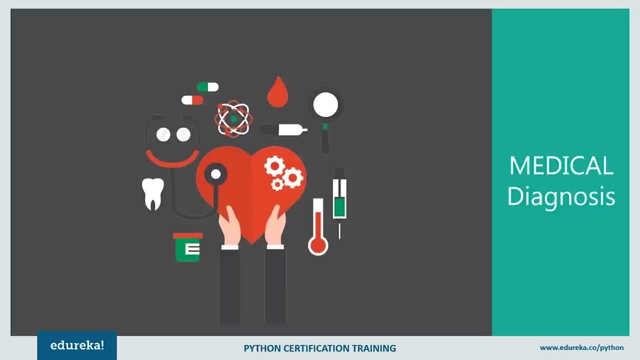 The produce medical data has certain characteristics that make their analysis very challenging and attractive as well. among all the different approaches, the naive bias is used. It is the most effective and the efficient classification algorithm and has been successfully applied to many medical problems. empirical comparison of naive bias versus five popular classifiers on 15 medical 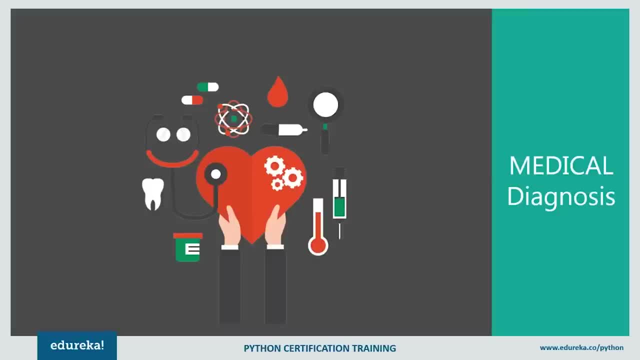 data sets shows that naive bias is well suited for medical application and has high performance in most of the examined medical problems. Now, in the past, various statistical methods have been used for modeling in the area of disease diagnosis. These methods require prior assumptions and are less capable of dealing. 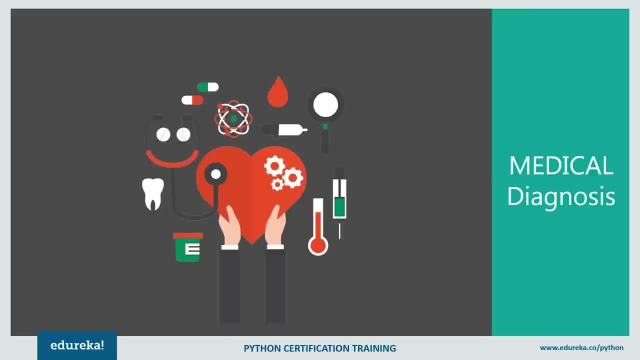 with massive and complicated nonlinear and dependent data. One of the main advantages of naive bias approach, which is appealing to Physicians, is that all the available information is used to explain the decision. this explanation seems to be natural for medical diagnosis and prognosis. that is, it is very close to the way how physician 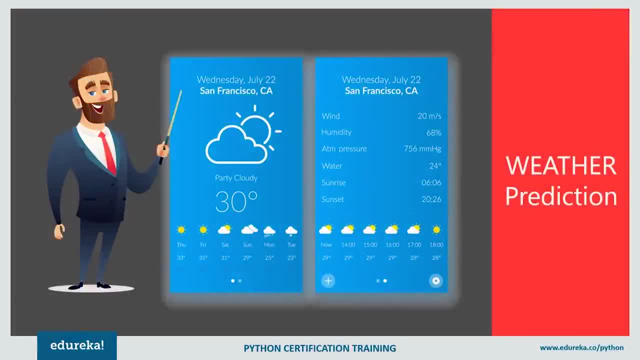 diagnose patients now whether is one of the most influential factor in our daily life, to an extent that it may affect the economy of a country that depends on occupation like agriculture. Therefore, as a countermeasure to reduce the damage caused by uncertainty in weather behavior, there should be an efficient way to predict the 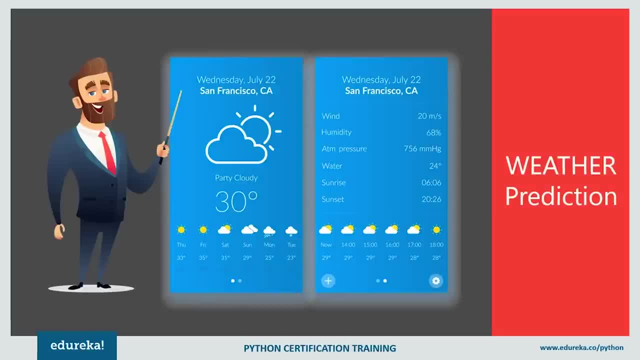 weather now. weather projecting has been challenging problem in the meteorological Department since years. even after the technological and scientific advancement, the accuracy in prediction of weather has never been sufficient. even in current date, This domain remains as a research topic in which scientists and mathematicians are working to produce a model or an algorithm that 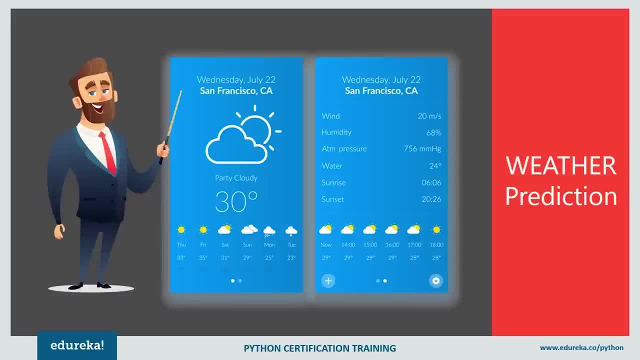 will accurately predict the weather. now a biasing approach based model is created by, where posterior probabilities are used to calculate the likelihood of each class label for input data instance, and the one with the maximum likelihood is considered as the resulting output. Now, earlier, we saw a small implementation of this algorithm as well. 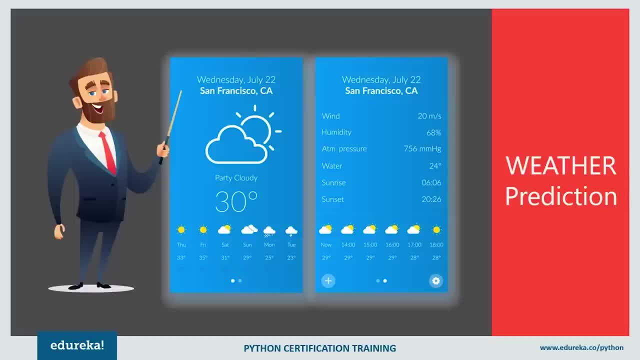 where we predicted whether we should play or not, based on the data which we have collected earlier. Now there is a python library which is known as scikit-learn. it helps to build naive bias and model in python. or there are three types of naive bias model under scikit-learn library. 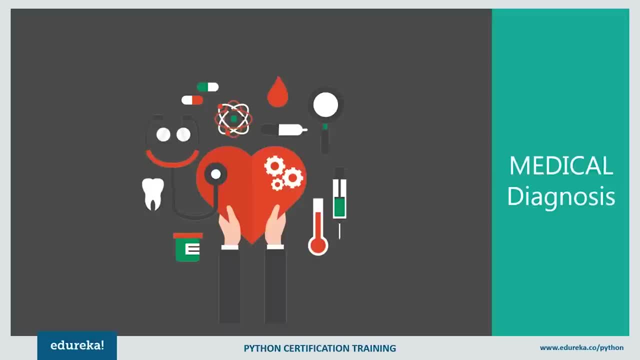 medical problems. empirical comparison of naive bias versus five popular classifiers on five popular classifiers is the most effective and the most effective method to inform the best assessment. now, the previous section of the video on naive bias versus five popular classifiers, which consists of 15 medical data sets, shows that naive bias is well suited for medical. 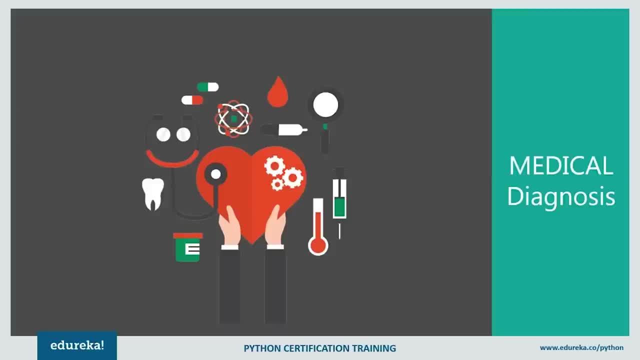 application and has high performance in most of the examined medical problems. now, in the past, various tactical methods have been used for modeling in the area of disease diagnosis. these methods require prior assumptions and are less capable of dealing with massive and complicated nonlinear and dependent data- one of the main advantages of naive bias approach, which is appealing to. 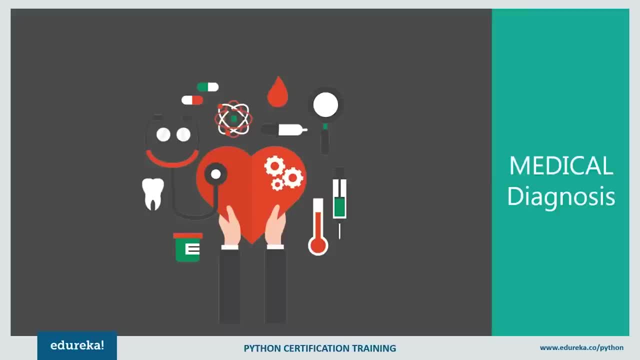 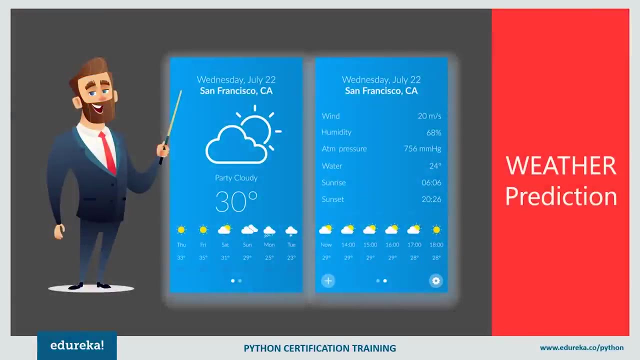 information is used to explain the decision. this explanation seems to be natural for medical diagnosis and prognosis. that is, it is very close to the way how physician diagnose patients. now, weather is one of the most influential factor in our daily life to an extent that it may affect the economy. 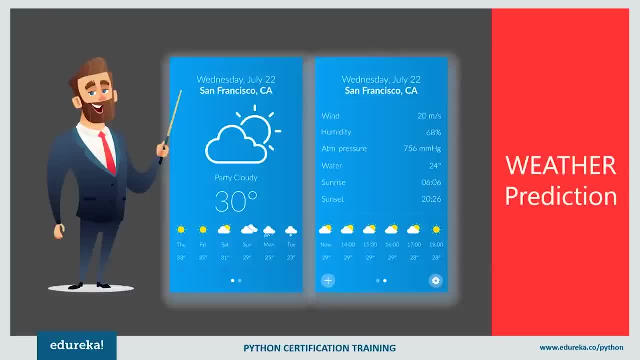 of a country that depends on occupation, like agriculture. therefore, as a countermeasure to reduce the damage caused by uncertainty in weather behavior, there should be an efficient way to predict the weather now. weather projecting has been challenging problem in the meteorological department since years. even after the technological and scientific advancement, the accuracy in 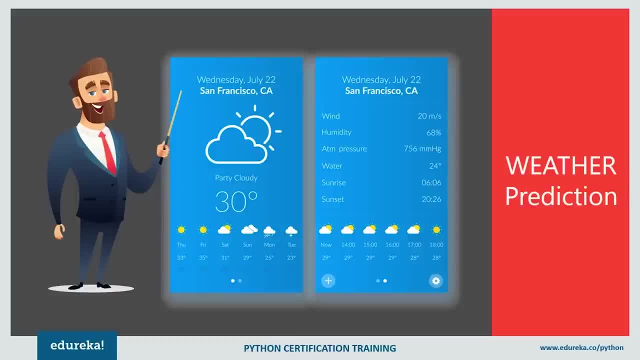 prediction of weather has never been sufficient, even in current date. this domain remains as a research topic in which scientists and mathematicians are working to produce a model or an algorithm that will accurately predict the weather. now, a biocene approach based model is created by where professionals and scientists are working to produce a model or an algorithm that will accurately predict the weather. now, a biocene approach based model is created by where 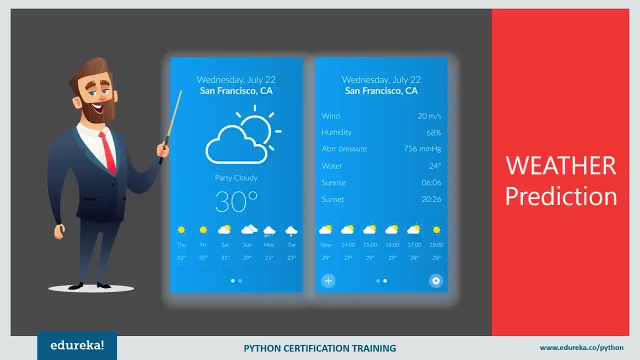 posterior probabilities are used to calculate the likelihood of each class label for input data instance, and the one with the maximum likelihood is considered as the resulting output. now, earlier we saw a small implementation of this algorithm as well, where we predicted whether we should play or not based on the data which we have collected earlier. now there is a Python. 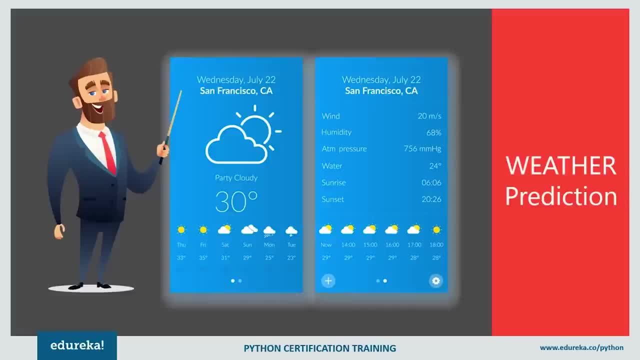 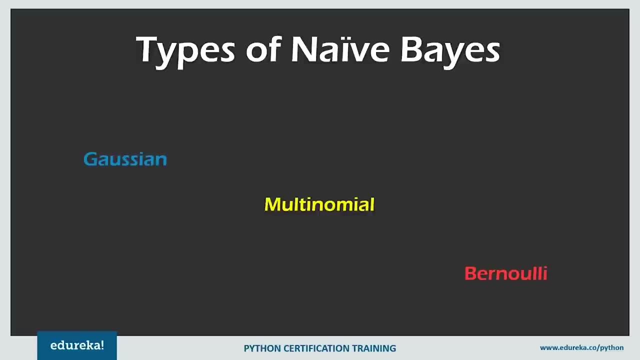 library, which is known as scikit-learn. it helps to build naive bias and model in Python. now there are three types of naive bias model under scikit-learn library. the first one is the caution. it is used in classification and it assumes that the feature follow a normal distribution. the next we have is: 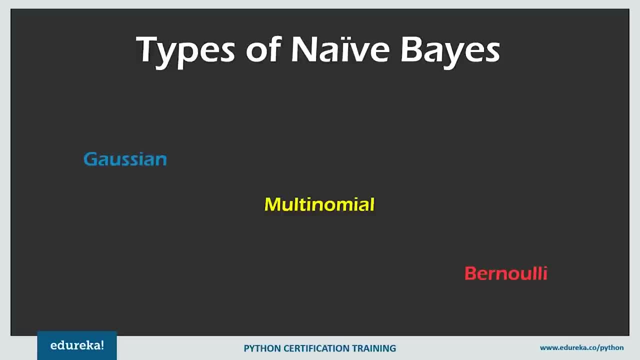 The first one is the Gaussian. it is used in classification and it assumes that the feature follow a normal distribution. the next we have is multinomial. It is used for discrete counts. For example, let's say we have a text classification problem and here we consider Bernoulli trials, which is one step further, and instead of 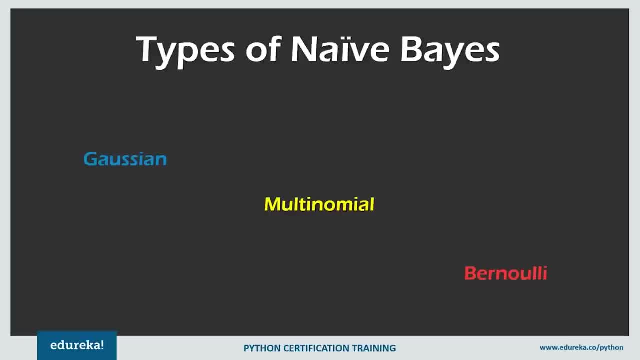 word occurring in the document. we have count how often word occurs in the document. you can think of it as- and the number of times outcomes number is observed in the given number of trials. and finally we have the Bernoulli type of naive bias. the binomial model is useful if your 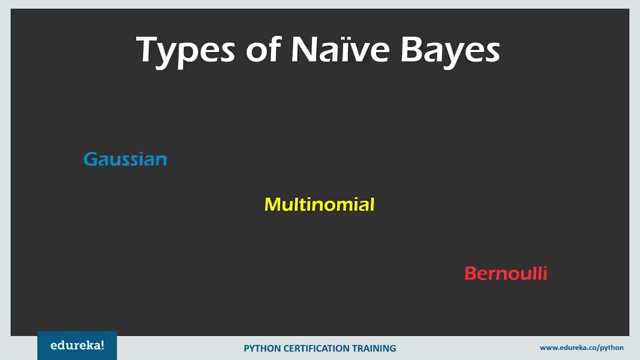 feature vectors are binary Bag of words model where the ones and the zeros are words occur in the document and the words which do not occur in the document, respectively based on their data set. You can choose any of the given discussed model here, which is the. 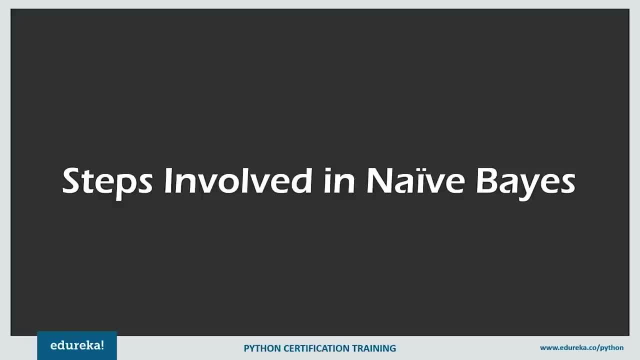 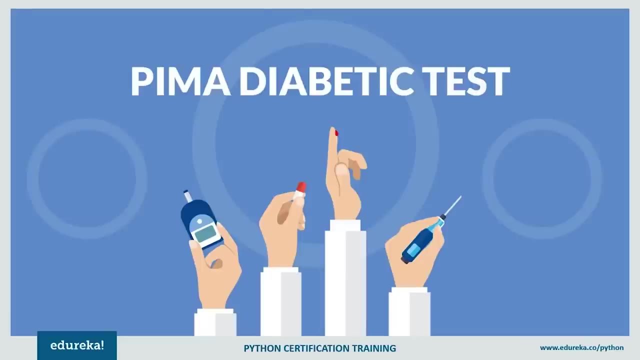 Gaussian, the multinomial or the Bernoulli. So let's understand how this algorithm works and what are the different steps one can take to create a Bayesian model and use naive bias to predict the output. So here to understand better, We are going to predict the onset of Diabetes. now this problem. 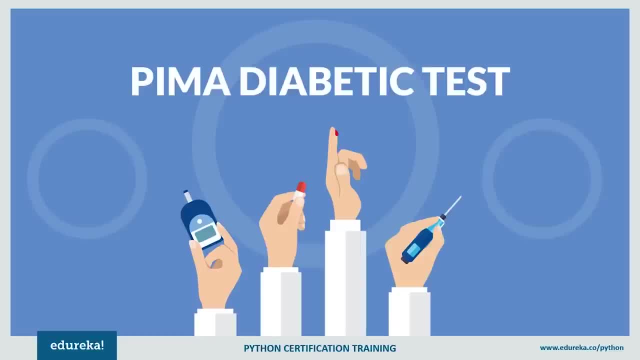 comprises of 768 observations of medical details for Pima Indian patients. the record describes instantaneous measurement taken from the patient, such as the age, the number of times pregnant and the blood work group. now, all the patients are women age 21 and older and all the attributes are numeric and the units vary from attributes. 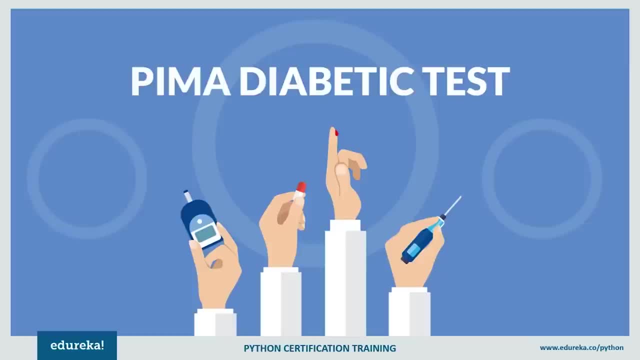 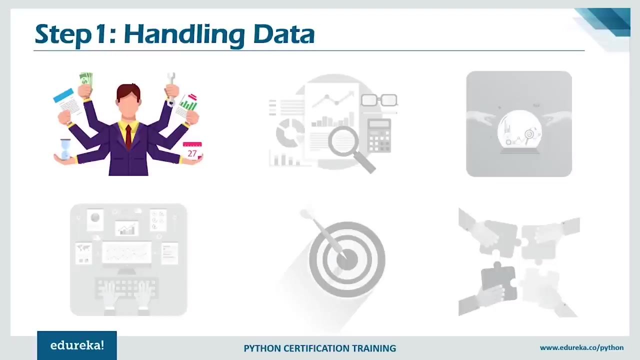 To attribute. each record has a class value that indicate whether the patient suffered on onset of Diabetes within five years, or the measurements. now these are classified as 0. now broken the whole process down into the following steps. The first step is handling the data in which we load the data from the 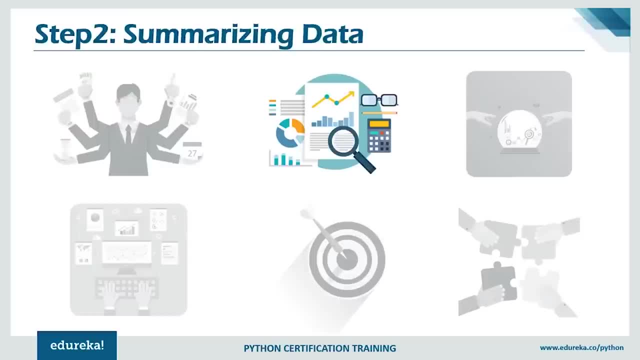 CSV file and spread it into training and test data sets. The second step is summarizing the data, in which we summarize the properties in the training data set so that we can calculate the probabilities and make predictions. Now the third step comes is making a particular prediction. 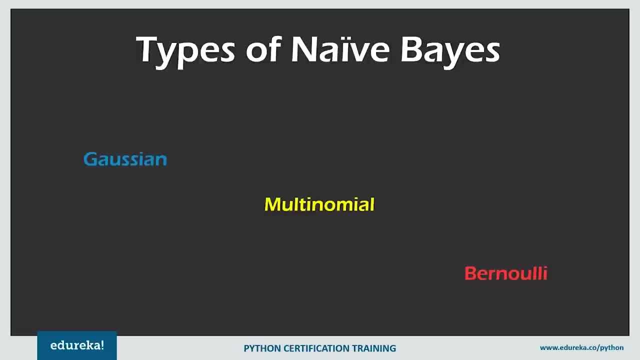 multinomial, it is used for discrete counts. for example, let's say we have a text classification problem, and here we consider Bernoulli trials, which is one step further, and instead of word occurring in the document, we have count how often word occurs in the document, you can think of it as- and the number of 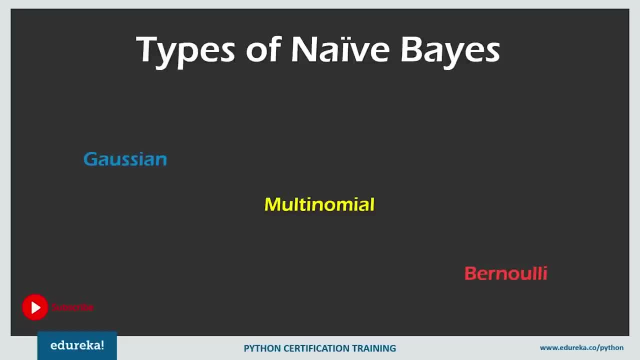 times outcomes number is observed in the given number of trials. and finally we have the Bernoulli type of nearby's. the binomial model is useful if your feature vectors are binary bag of words model, where the ones and the zeros are words occur in the document and the 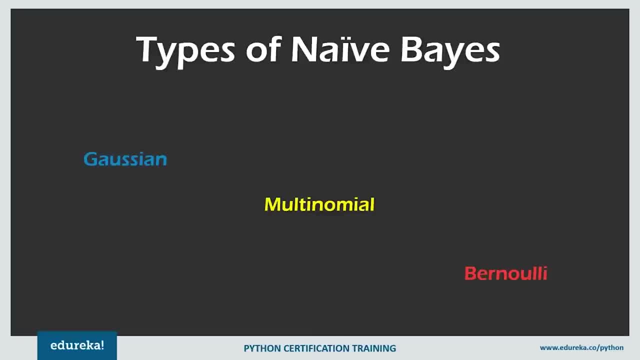 words which do not occur in the document, respectively based on their data set, you can choose any of the given discussed model here, which is the Gaussian, the multinomial or the Bernoulli. so let's understand how this algorithm works and what are the different steps one can take to create a Bajan model and use. 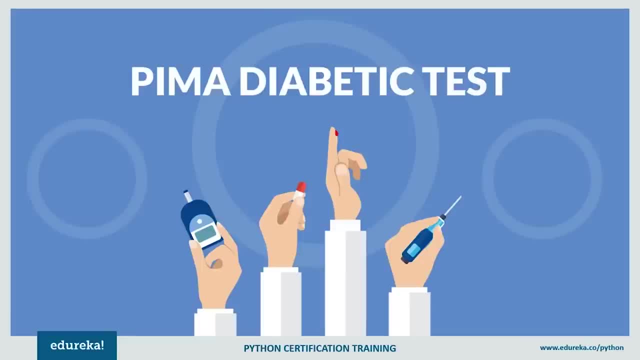 need bias to predict the output. so here, to understand better, we are going to predict the onset of diabetes now. this problem comprises of 768 observations of medical details for Pima Indian patients. the record describes instantaneous measure of the relation between the information of the motivation to the. 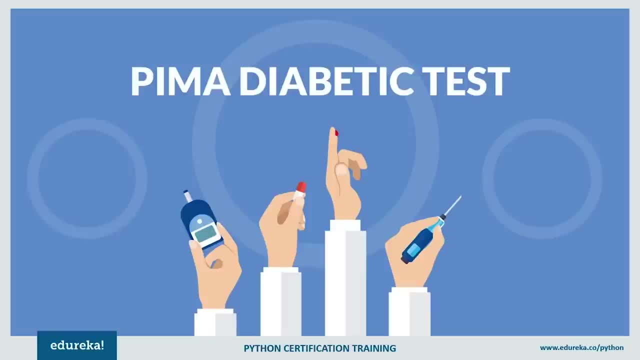 measurement taken from the patients, such as their age, the number of times pregnant and the blurred work group. Now all the patients are women age 21 and older and all the attributes are numeric and the units vary from attribute to attribute. Each record has a class value that indicate. 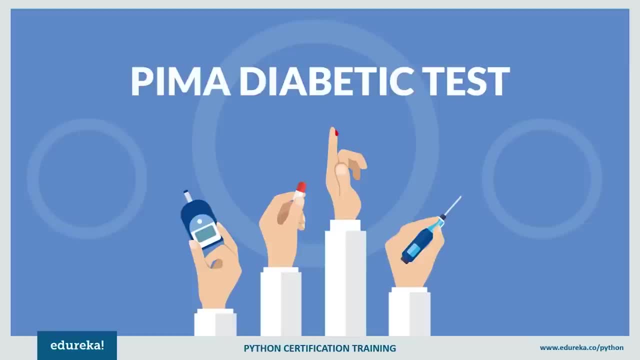 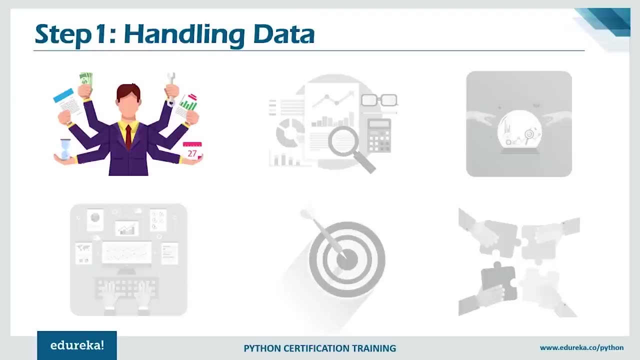 whether the patient suffered on onset of diabetes within five years or the measurements. Now these are classified as 0.. Now I've broken the whole process down into the following steps. The first step is handling the data, in which we load the data from the CSV file and split it into training. 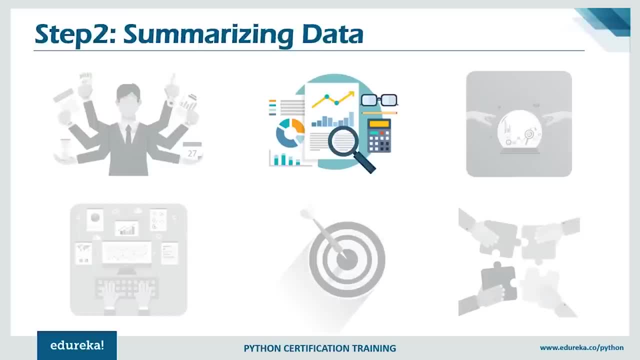 and test data sets. The second step is summarizing the data, in which we summarize the properties in the training data sets so that we can calculate the probabilities and make predictions. Now the third step comes is making a particular prediction. We use the summaries of the data set to generate a 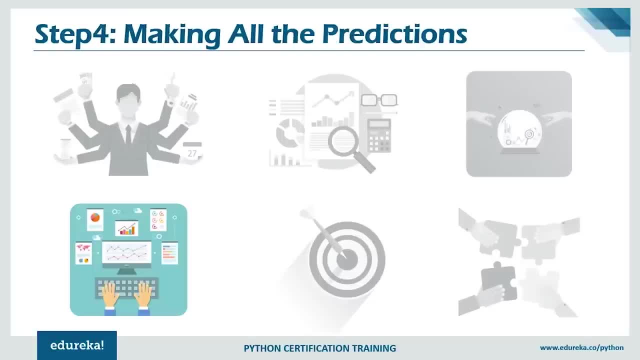 We use the summaries of the data set to generate a single prediction and after that we generate predictions given a test data set and a summarized training data sets. and finally we evaluate the accuracy of the predictions made for a test data set as a percentage correct out of all the predictions made and finally we tie it together and form. 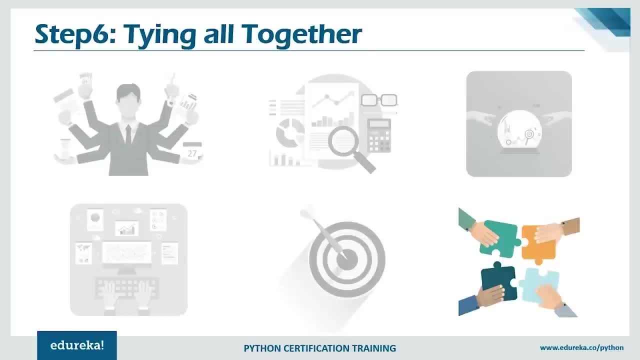 our own model of naive bias classifier. But the first thing we need to do is load our data. The data is in the CSV format without a header line or any quotes. We can open the file with the open function and read the data lines using the read functions in the CSV module. 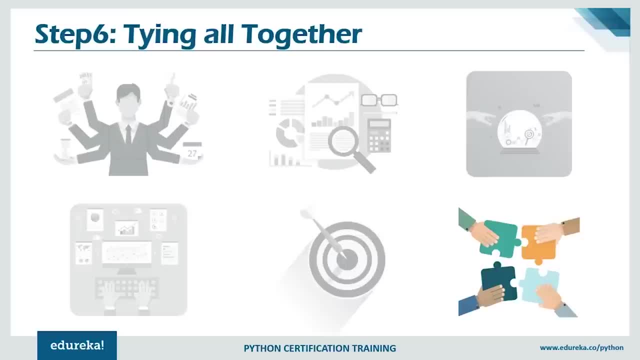 Now we also need to convert the attributes that were loaded as strings into numbers so that we can work with them. So let me show you how this can be implemented. for that you need to install python on your system and use the Jupiter notebook or the 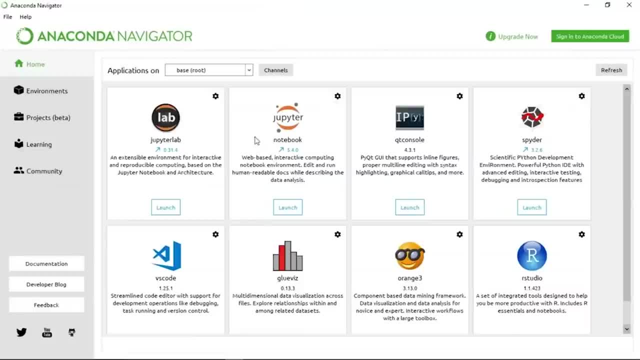 python shell. Hey, I'm using the anaconda Navigator, which has all the things required to do programming in python. We have the Jupiter lab, We have the notebook, We have the QT console, even we have a studio as well. So what you need to do is just install the anaconda Navigator. 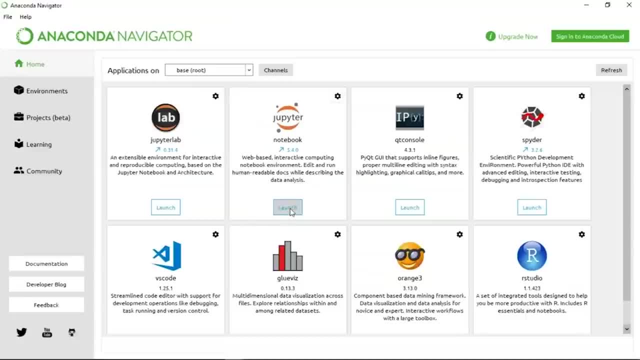 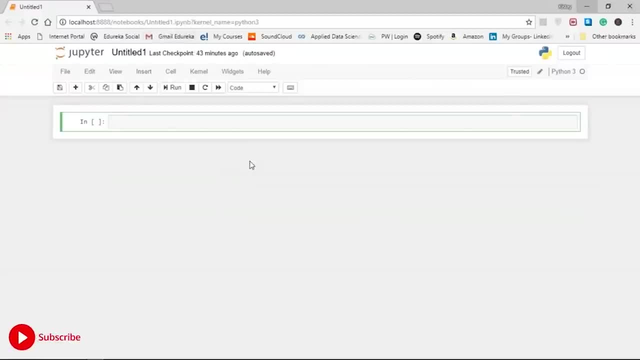 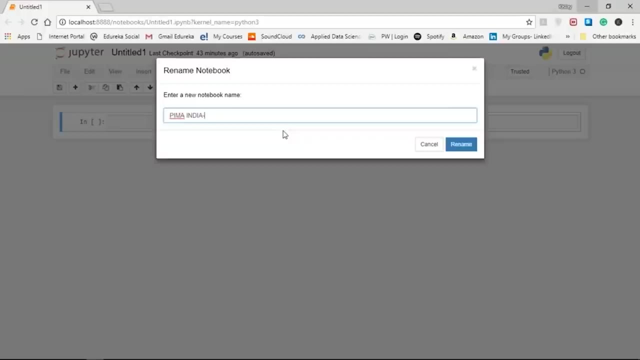 It comes with the pre-installed python also. So the moment you click launch on the Jupiter notebook, it will take you to the Jupiter home page in a local system and here you can do programming in python. So let me just rename it as by my: India: diabetes. 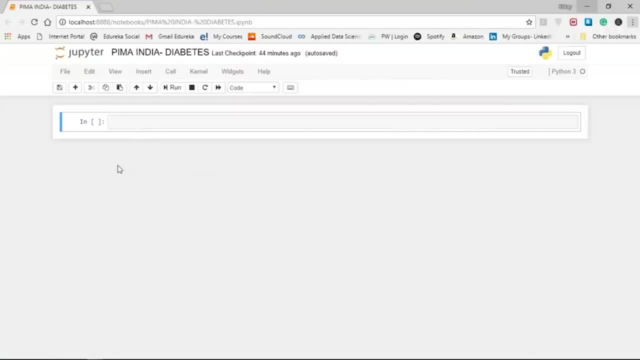 So first we need to load the data set. So I'm creating here a function: load CSV. Now, before that, we need to import certain CSV, the math and the random method. So, as you can see, I've created a load CSV function which will take. 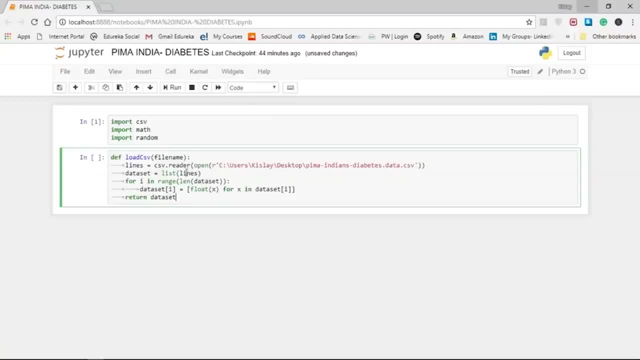 the Pima Indian diabetes data dot CSV file using the CSV dot reader method. And then we are converting every element of that data set into float. originally all the elements are in string, but we need to convert them into float for all calculation purposes. The next: we need to split the data into training data sets. that 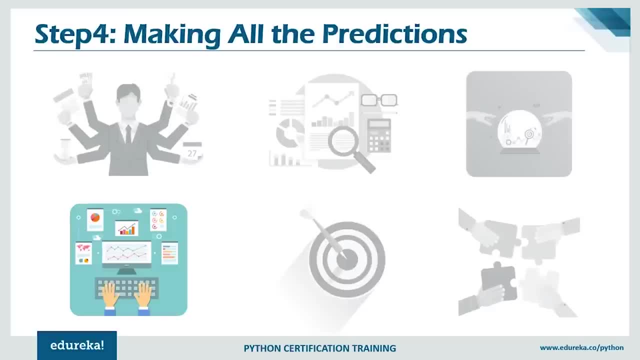 single prediction and after that we generate predictions given a test data set and a summarize training data sets and finally we evaluate the accuracy of the predictions made for a test data set as the percentage correct out of all the predictions made and finally we tie it together and form our own model of Nape Viase. 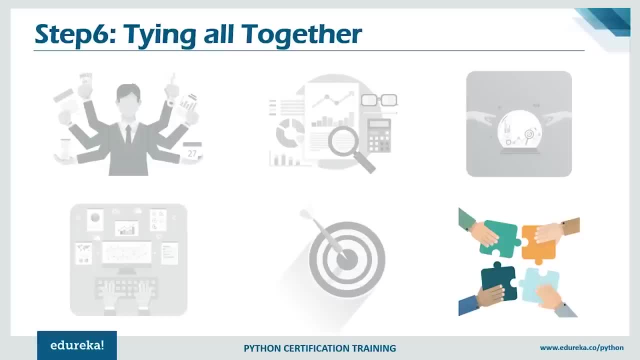 Classifier. Now the first thing we need to do is load our data. The data is in the CSV format without a header line or any quotes. We can open the file with the open function and read the data lines using the CSV file. Now, if we open the file with the open function and read the data lines, 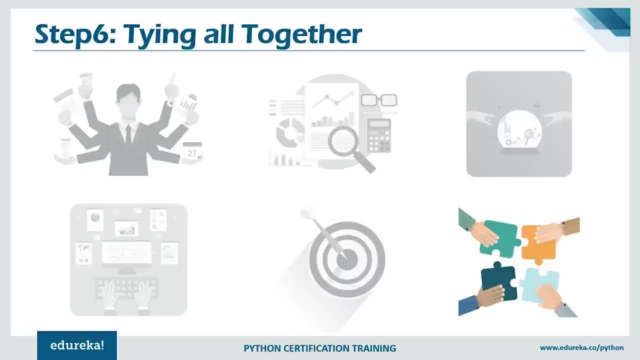 using the open function and read the data lines using the CSV file. we can open the file with the the read functions in the CSV module. now we also need to convert the attributes that were loaded as strings into numbers so that we can work with them. so let me. 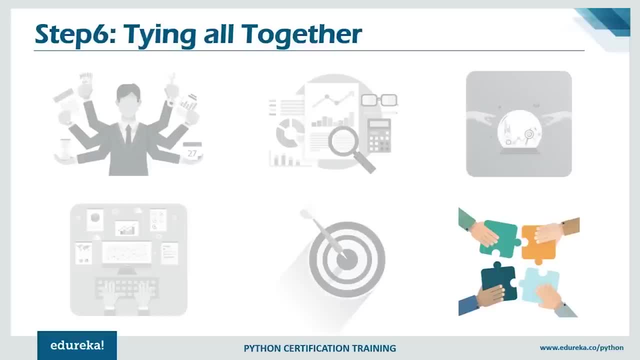 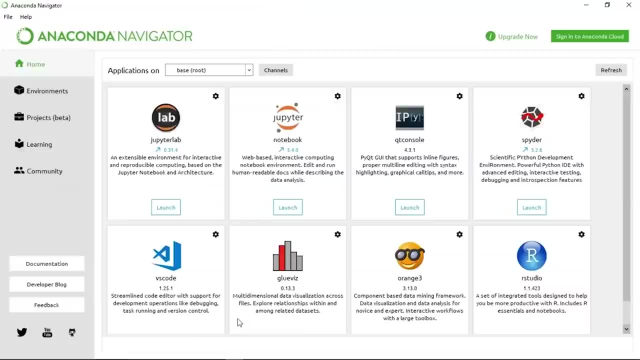 show you how this can be implemented now. for that you need to install Python on your system and use the Jupyter notebook or the Python shell. here I am using the anaconda navigator, which has all the things required to do programming in Python. we have the Jupyter lab, we have the notebook, we have the Qt console, even. 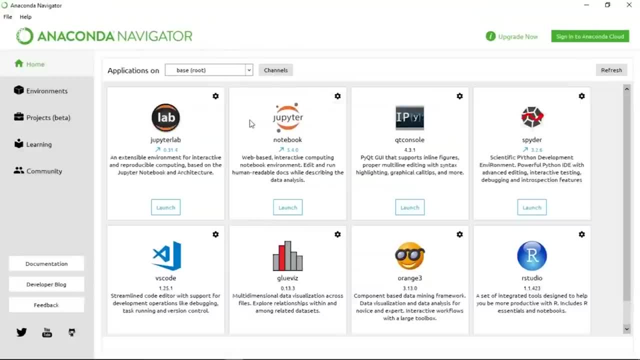 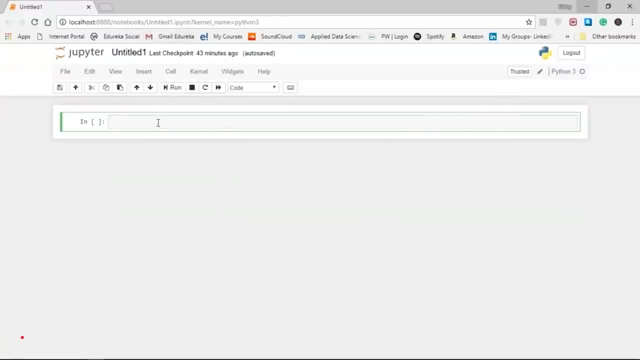 we have R studio as well, so what you need to do is just install the anaconda navigator. it comes with the pre-installed Python also, so the moment you click launch on the Jupyter notebook, it will take you to the Jupyter homepage in a local system and here you can do programming in Python. so let me just 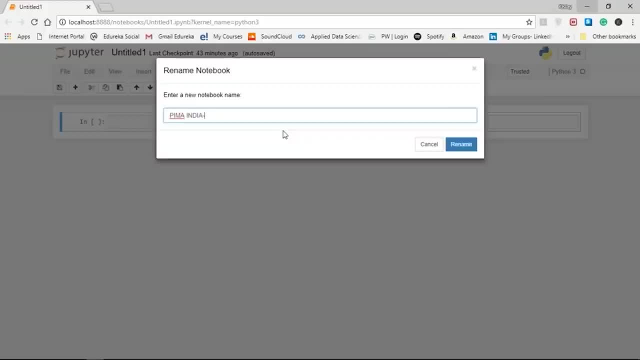 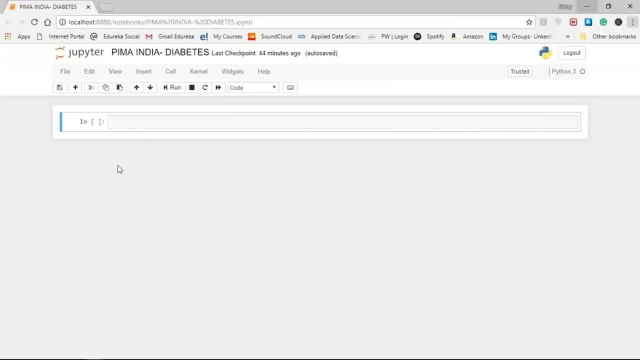 rename it as by my India diabetes you. so first we need to load the data set. so I'm creating here a function: load CSV. now, before that we need to import certain CSV, the math and the random method. so, as you can see, I've created a load CSV function which will take the 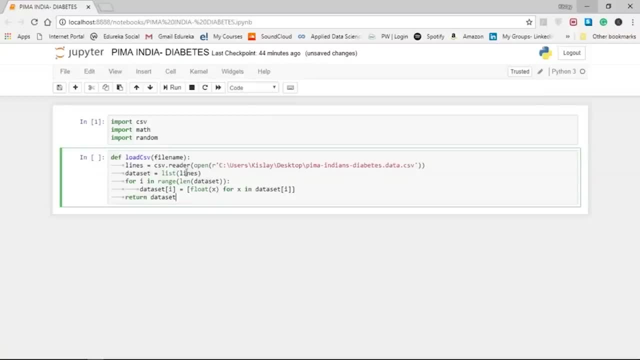 Pima Indian diabetes data dot CSV file using the CSV dot reader method. and then we are converting every element of that data set into float originally: all the, you. the data set into float originally, all the. the data set into float originally, all the. the data set into float originally, all the. 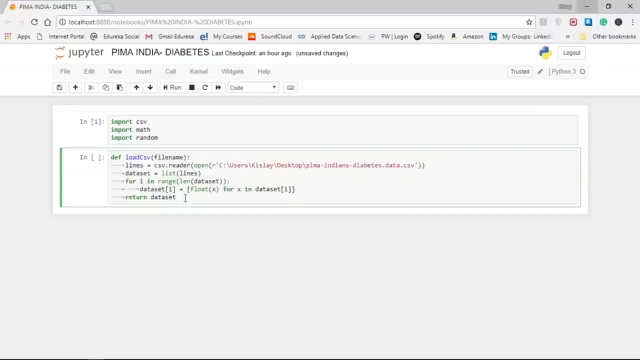 elements are in string, but we need to convert them into float for all calculation purposes. now, next, we need to split the data into training data sets that nape bias can use to make the prediction and test data set that we can use to evaluate the accuracy of the model. we need to split the data set. 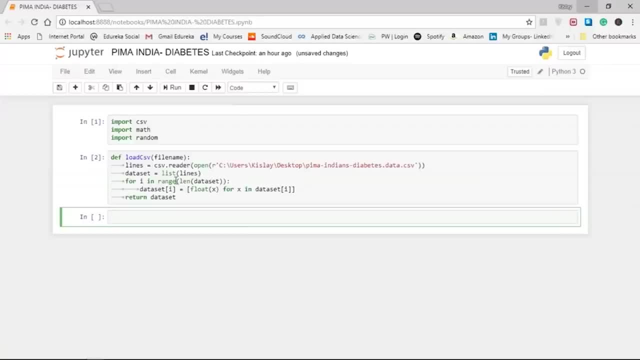 naive bias can use to make the prediction and test data set that we can use to evaluate the accuracy of the model. We need to split the data set randomly into training and testing data set in the ratio Of usually, which is 70 to 30.. 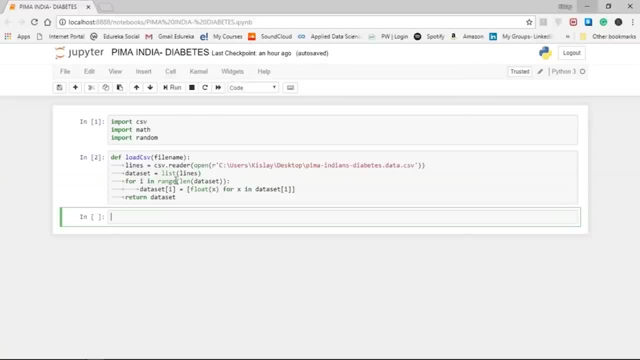 But for this example, I'm going to use 67 and 33. now, 70 and 30 is a common ratio for testing algorithms, So you can play around with this number. So this is our split data set function. Now, the naive bias model is comprised of summary of the data in the 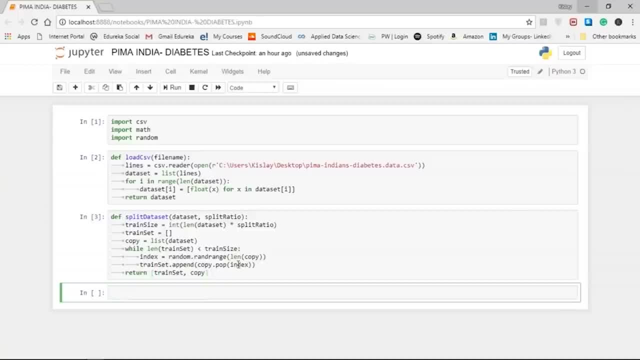 training data set. Now. this summary is then used while making predictions. Now, the summary of the training data collected involves the mean, the standard deviation Of each attribute by class value. Now, for example, if there are two class values and seven numerical attributes, then we need a mean and the standard deviation for each. 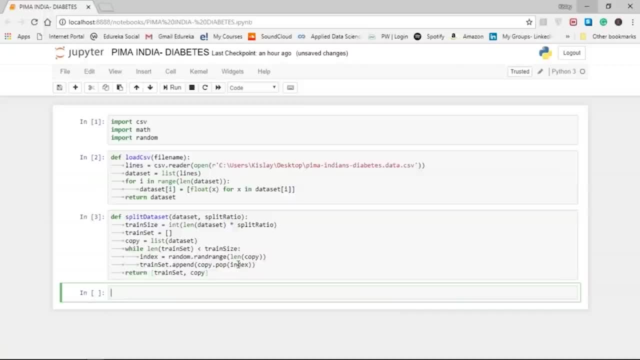 of these seven attributes and the class value which makes it the 14 attribute summaries. So we can break the preparation of this summary down into the following subtasks, which are the separating data by class, calculating mean, calculating standard deviation, summarizing the data sets and 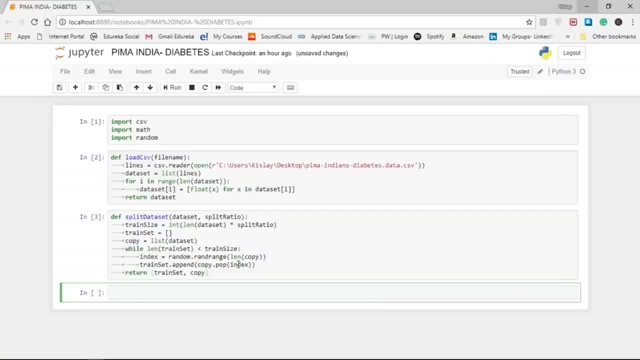 summarizing attributes by class. So the first task is to separate the training data set instances by class value so that we can calculate statistics for each class. We can do that by creating a map of each class value to a list of instances that belong to the class and sort the entire data set of 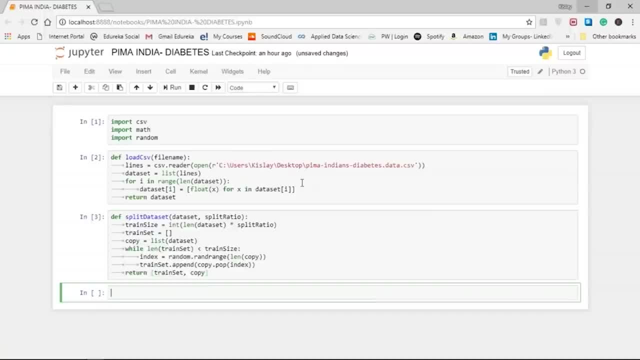 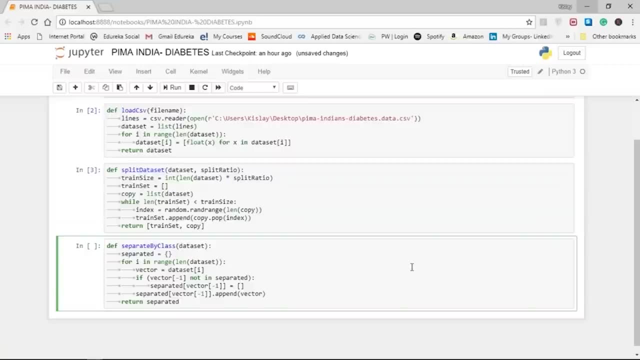 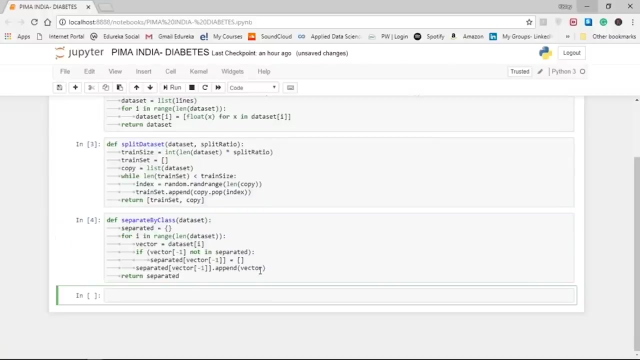 instances into the appropriate list. Now the separate by class function just does the same. So, as you can see, the function assumes that the last attribute is the class value. the function returns a map of class Class value to the list of data instances. Next we need to calculate the mean of each attribute for a class. 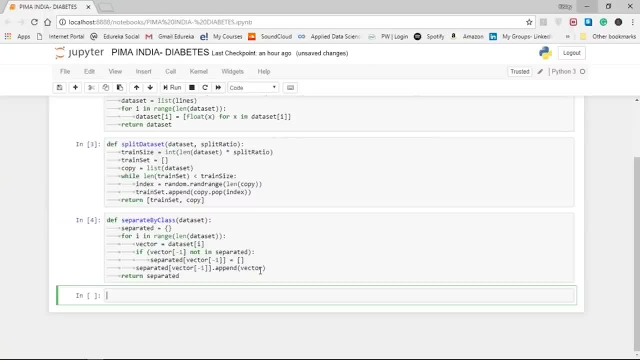 value. Now the mean is the central middle or the central tendency of the data, and we use it as a middle of our Gaussian distribution when calculating the probabilities. So this is our function. for me Now we also need to calculate the standard deviation of each. 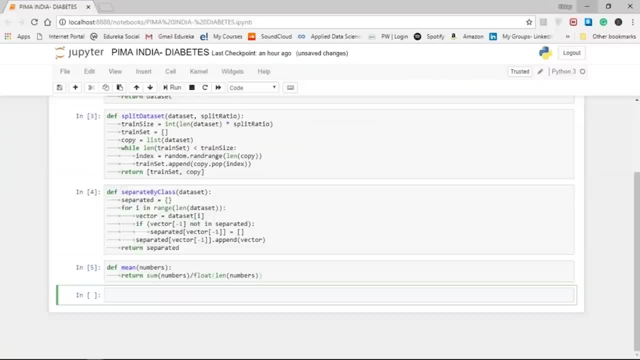 attribute for a class value. The standard deviation is calculated as a square root of the variance, and the variance is calculated as the average of the square Differences for each attribute value from the mean. Now, one thing to note that here is that we are using n minus 1 method. 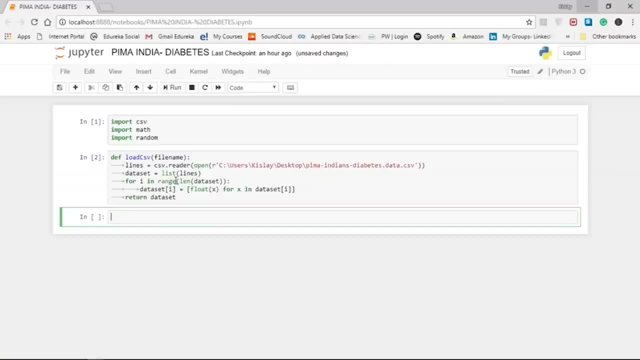 randomly into training and testing data set in the ratio of usually, which is 70 to 30, but for this example, I am going to use 67 and 33. now, 70 and 30 are the data is a common ratio for testing algorithms, So you can play around with this number. 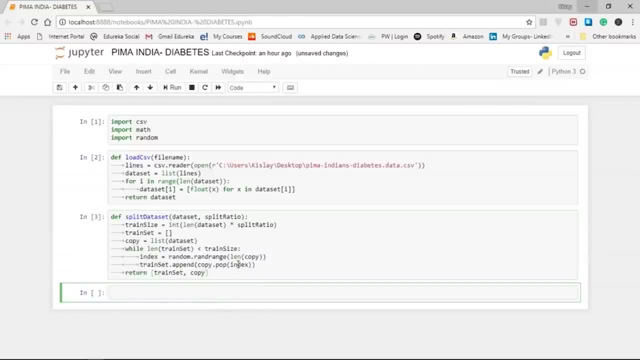 So this is our split data set function. Now the naive bias model is comprised of summary of the data in the training data set. Now this summary is then used while making predictions. Now, the summary of the training data collected involves the mean, the standard deviation of each attribute. 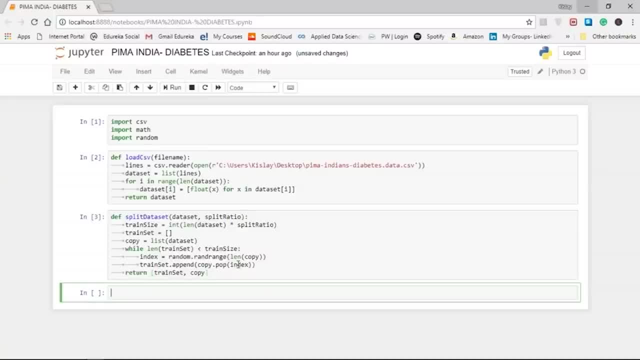 by class value. Now, for example, if there are two class values and seven numerical attributes, then we need a mean and the standard deviation for each of these seven attributes and the class value which makes it the 14 attribute summaries. So we can break the preparation of this summary. 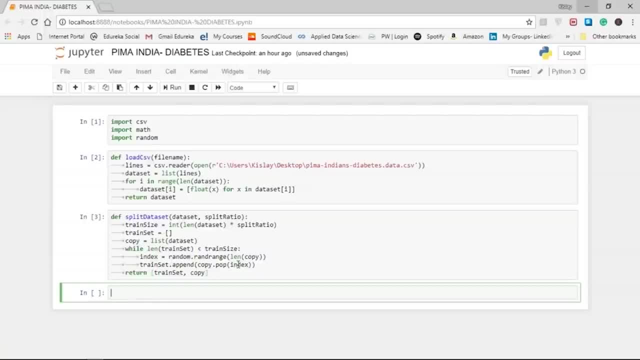 down into the following subtasks, which are the: separating data by class, calculating mean, calculating standard deviation, summarizing the data sets and summarizing attributes by class. So the first task is to separate the training data set instances by class value, so that we 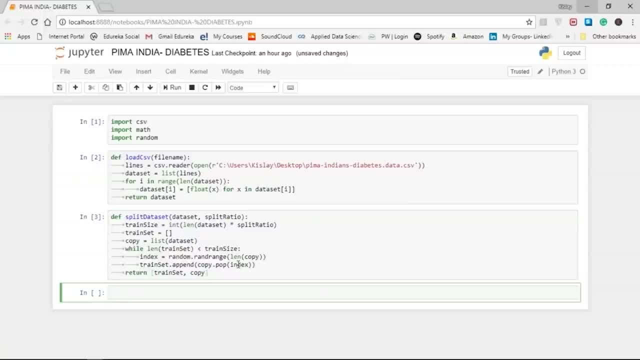 can calculate statistics for each of the attributes. So the first task is to separate the training data set instances by class. We can do that by creating a map of each class value to a list of instances that belong to the class and sort the entire data set of instances into the appropriate 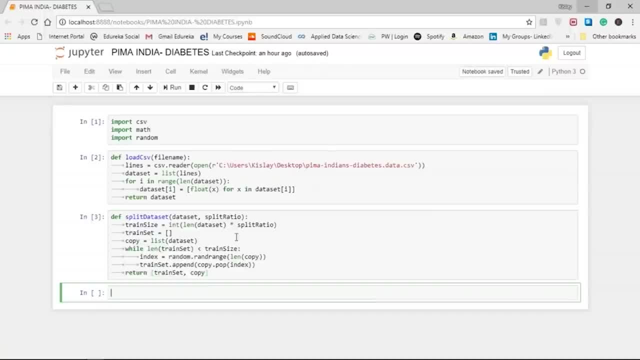 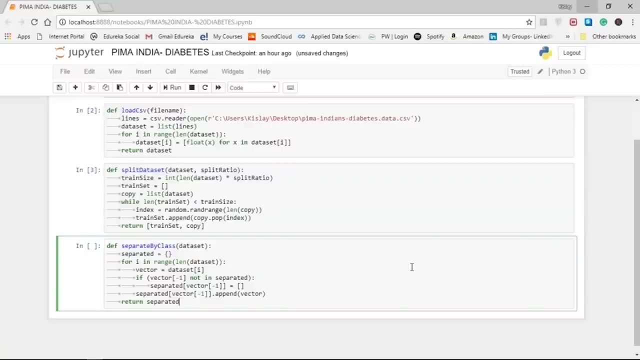 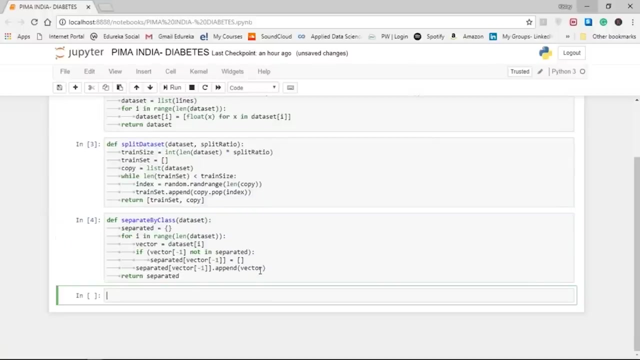 list. Now the separate by class function just does the same. So, as you can see, the function assumes that the last attribute is the class value. The function returns a map of class value to the list of data instances. Next we need to calculate the mean of each attribute for a class value. 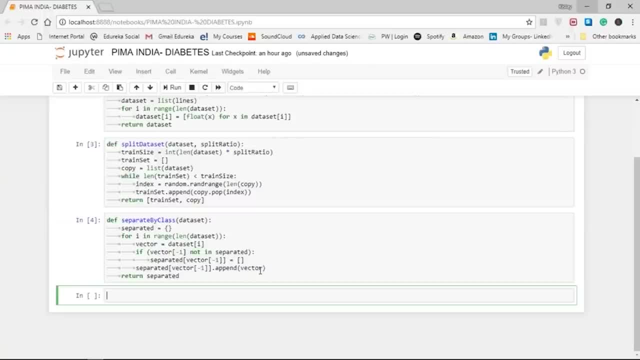 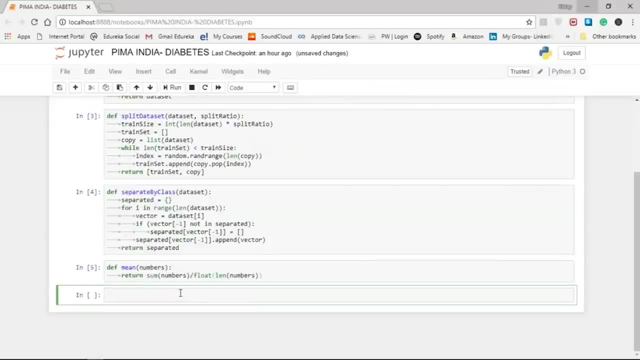 Now the mean is the central middle or the central tendency of the data, and we use it as the middle of our Gaussian distribution when calculating the probabilities. So this is our function for mean. Now we also need to calculate the standard deviation of each attribute for a class value. 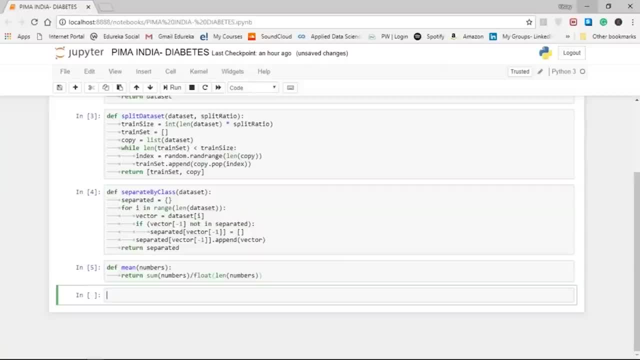 The standard deviation is calculated as a square root of the variance and the variance is calculated as the average of the square differences for each attribute value from the mean. Now, one thing to note that here is that we are using the standard deviation of each attribute for a class value. 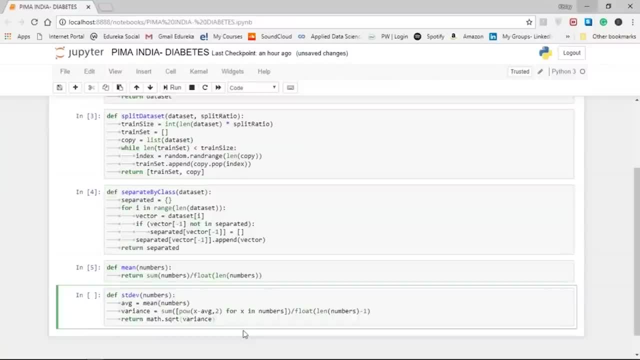 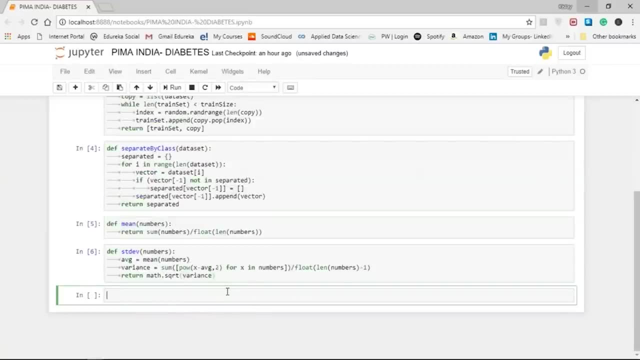 We are using the n-1 method, which subtracts one from the number of attributes values when calculating the variance. Now that we have the tools to summarize the data for a given list of instances, we can calculate the mean and standard deviation for each attribute. Now the zip function groups: 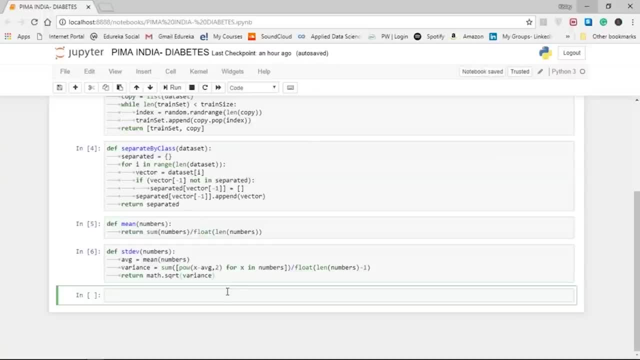 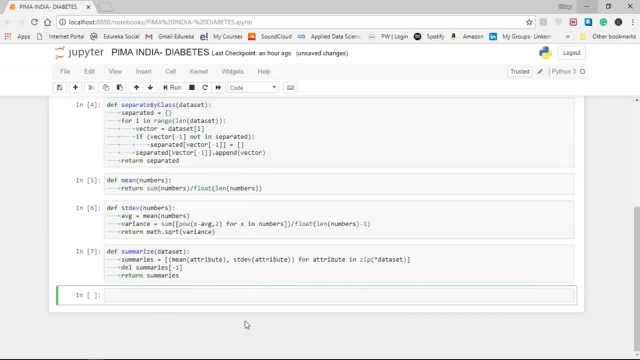 the values for each attribute across our data instances into their own list, so that we can compute the mean and standard deviation values for each attribute. Now next comes the summarizing attributes by class. We can pull it all together By first separating our training data sets into instances grouped by class, then calculating the 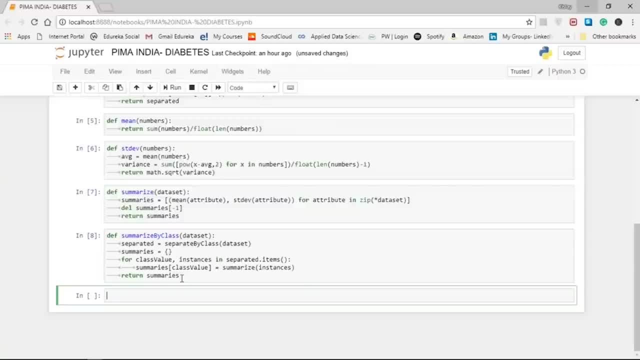 summaries for each attribute. Now we are ready to make predictions using the summaries prepared from our training data. Making predictions involved calculating the probability that a given data instance belongs to each class, then selecting the class with the largest probability as a prediction. Now we can divide this whole method into four tasks, which are the calculating Gaussian probability. 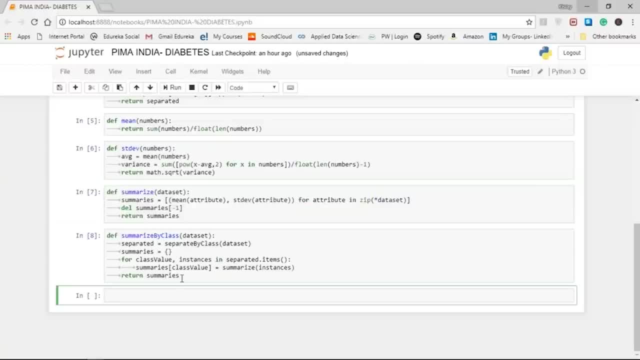 density function: calculating class probability, making a prediction and then estimating the accuracy. Now to calculate the Gaussian probability density function. we use the Gaussian function to estimate the probability of a given attribute value, given the known mean and the standard deviation of the attribute estimated from the training data. As you can see, the parameters are x mean and the standard. 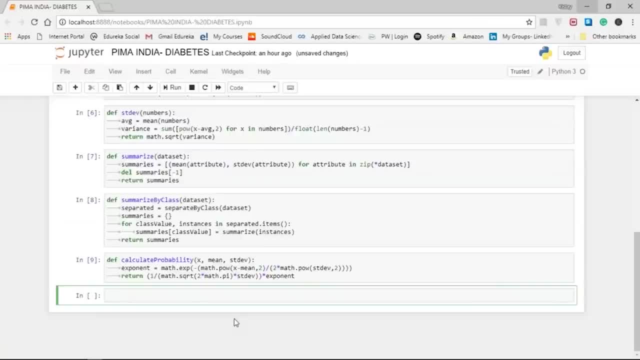 deviation. Now in the calculate probability function we calculate the exponent first, then calculate the main division. This lets us fit the equation nicely into two lines. now the next task is calculating the class probabilities. Now that we can calculate the probability of an attribute belonging to a class, we can combine the probabilities of all the attributes values. 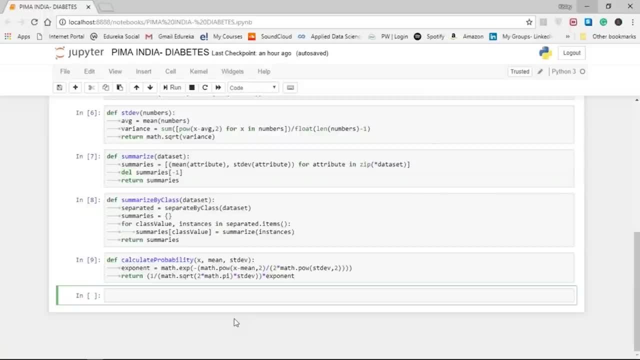 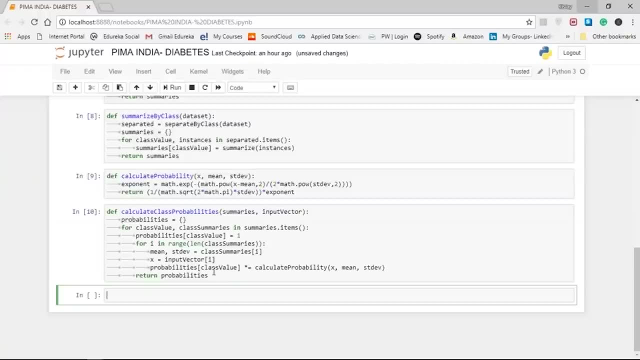 for a data instance And come up with the probability of the entire data instance belonging to the class. Now that we have calculated the class probabilities, it's time to finally make our first prediction- the probability of the data instance belonging to each class value- and we can look for the largest probability. 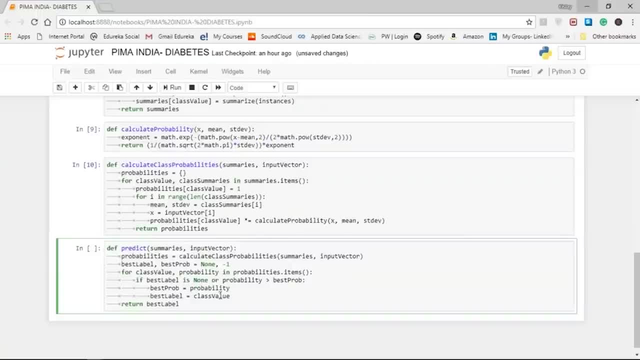 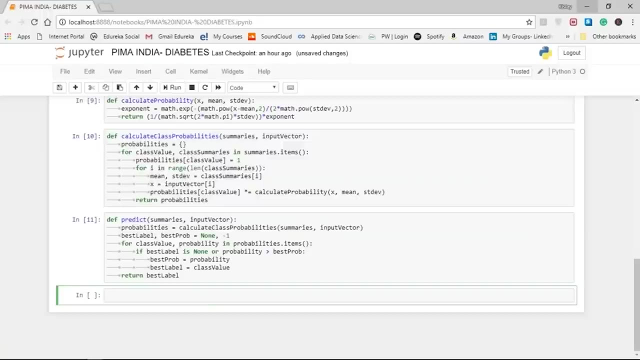 and return the associated class, and for that we are going to use this function predict, which uses the summaries and the input vector, which is basically all the probabilities which are being input for a particular label. Now, finally, we can estimate the accuracy of the model by making predictions for each data instances in our test data. 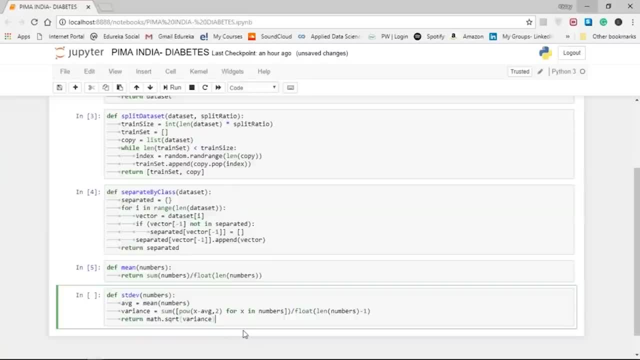 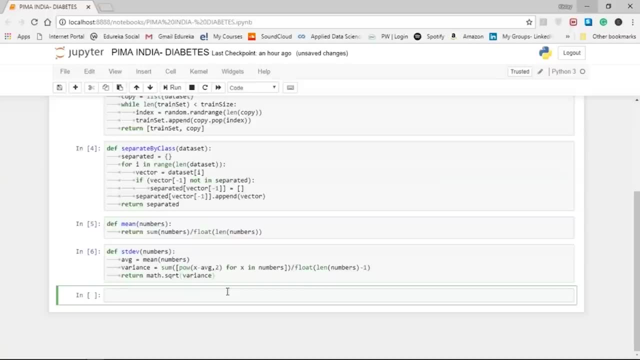 which subtracts 1 from the number of attributes values. when calculating the variance, And now that we have the tools to summarize the data for a given list of instances, we can calculate the mean and standard deviation for each attribute. Now, that's if function groups the values for each attribute across. 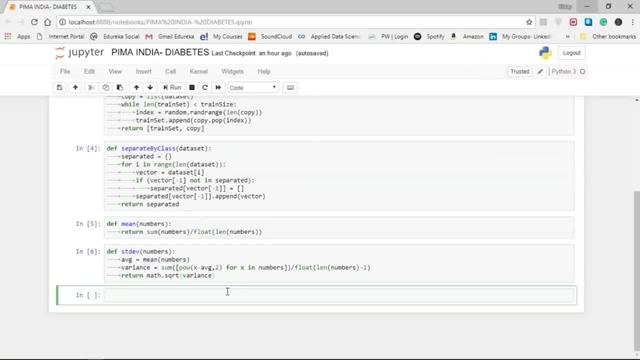 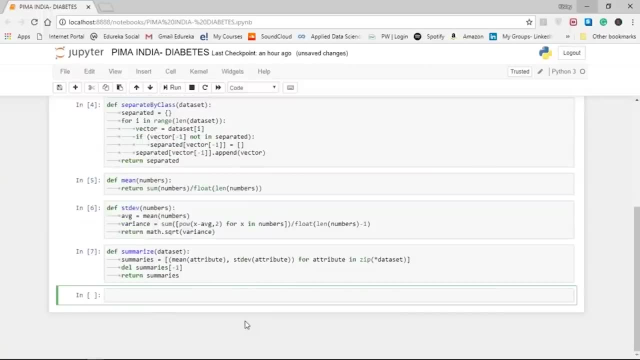 our data instances into their own list so that we can compute the mean and standard deviation values for each attribute. The next comes to summarizing attributes by class. We can pull it all together by first separating our training data sets into instances- growth by class, then calculating the 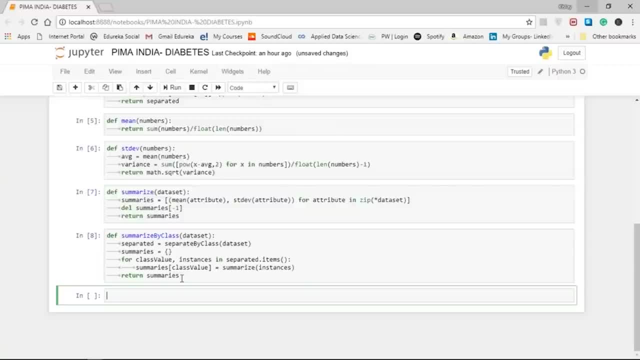 summaries for each attribute. Now we are ready to make predictions using the summaries prepared from our training data. making predictions involved calculating the probability that a given data instance belong to each class, then selecting the class with the largest probability as the prediction. Now we can divide this whole method into four tasks, which are: 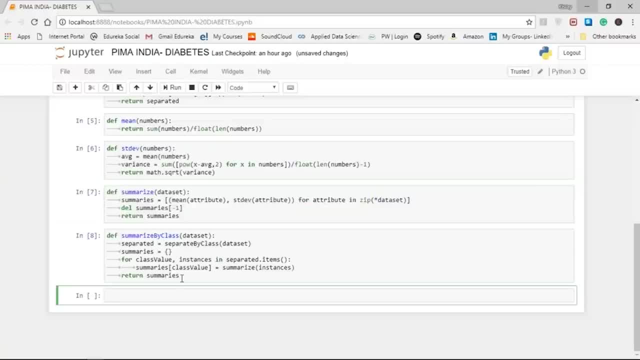 the calculating Gaussian probability density function, calculating class probability, making a prediction and then estimating the accuracy. Now to calculate the Gaussian probability density function. We use the Gaussian function to estimate the probability of a given attribute value, given the node mean and the standard deviation of the attribute estimated from the training data. 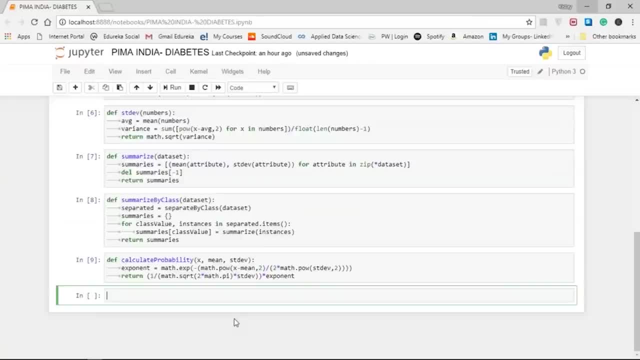 As you can see, the parameters are X, mean and the standard deviation. Now in the calculate probability function, We calculate the exponent first, then calculate the main division. this lets us fit the equation nicely into two lines. Now the next task is calculating the class properties. now that 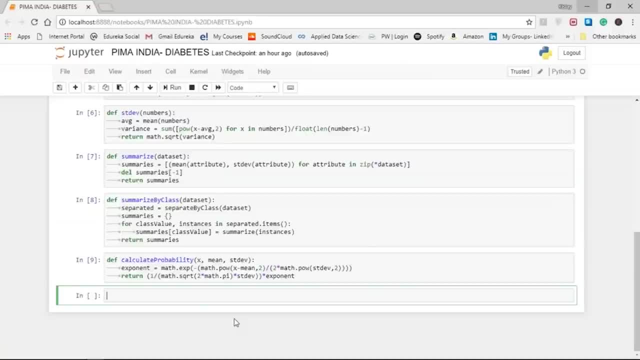 we can calculate the probability of an attribute belonging to a class. we can combine the probabilities of all the attributes values for a data instance and come up with a probability of the entire data instance Belonging to the class. So now that we have calculated the class properties, it's time. 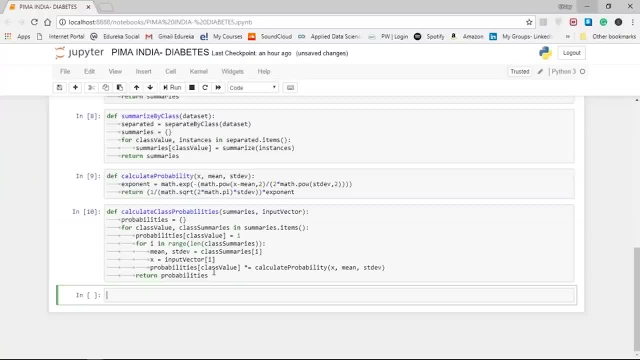 to finally make our first prediction. Now we can calculate the probability of the data instance belonging to each class value and we can look for the largest probability and return the associated class, and for that we are going to use this function predict, which uses the summaries. 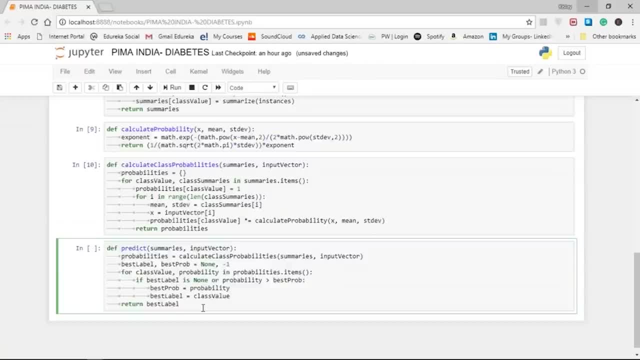 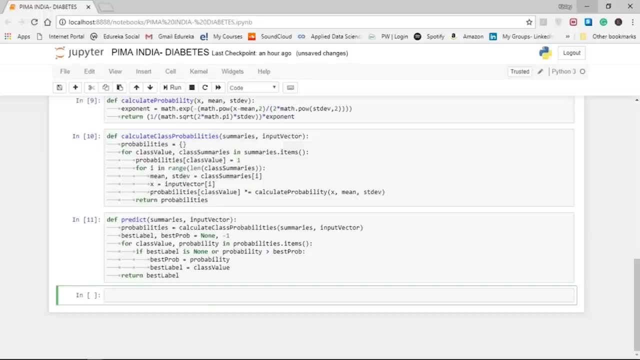 and the input vector, which is basically all the probabilities which are being input for a particular label. Now, Finally, we can estimate the accuracy See of the model by making predictions for each data instances in our test data. for that we use the get predictions method. 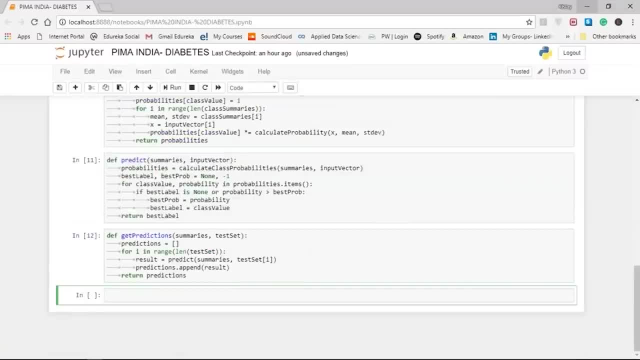 Now this method is used to calculate the predictions based upon the test data sets and the summary of the training data set. Now the predictions can be compared to the class values in our test data set, and classification accuracy can be calculated as an accuracy ratio between the zeros and the hundred percent. 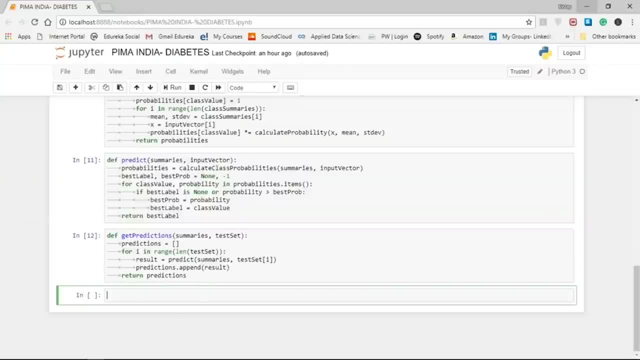 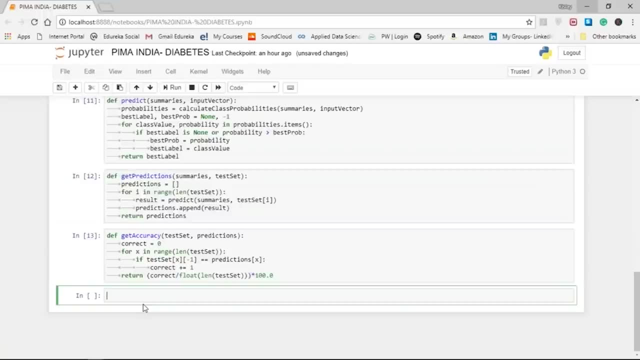 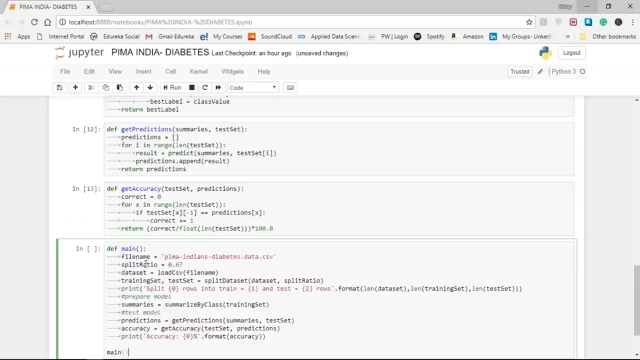 Now the get accuracy method will calculate this accuracy ratio. Now, finally, to sum it all up, We define our main function. We call all these methods which we have defined earlier, one by one, to get the accuracy of the model which we have created. So, as you can see, this is our main function, in which we have 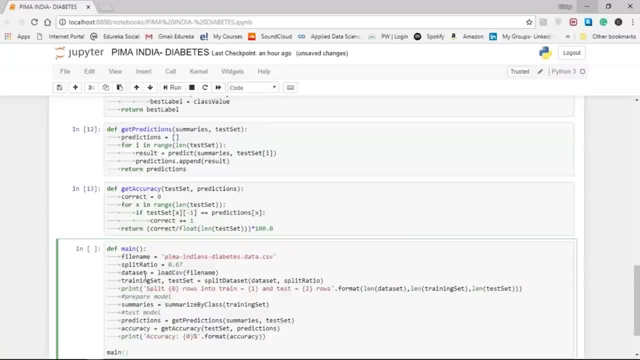 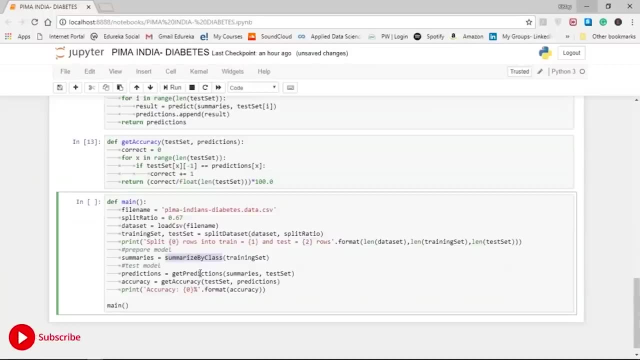 the file name. We have to define the split ratio. We have the data set. We have the training and test data set. We are using the split data set method. next, We are using the summarized by class function. We are using the get prediction and the get accuracy method as well. 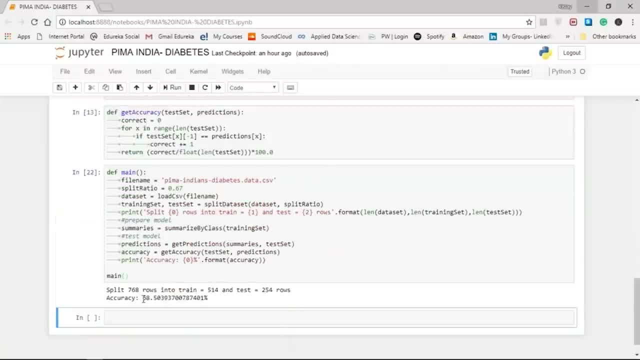 So, guys, as you can see, the output of this one gives us that we are splitting the 768 rows into 514,, which is the training, and 254,, which is the test data set rows, and the accuracy of this model is 68%. now we can play with the amount of training and test data. 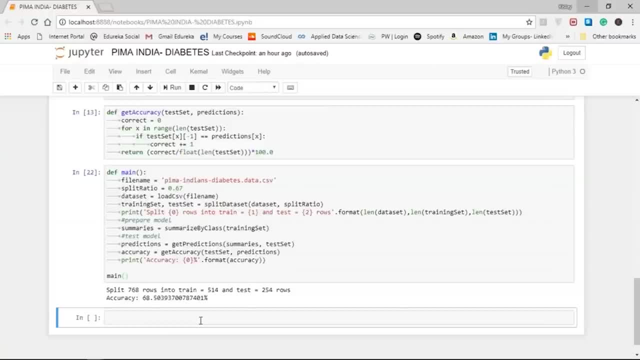 sets which are to be used here, so we can change the split ratio to 70s to 30, 80s to 20 to get different sort of accuracy. So suppose I change the split ratio from 0.67 to 0.8.. 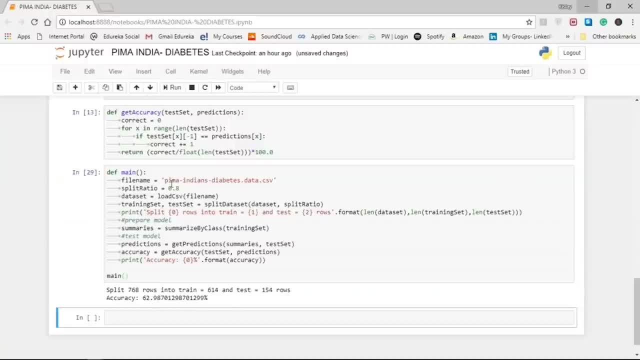 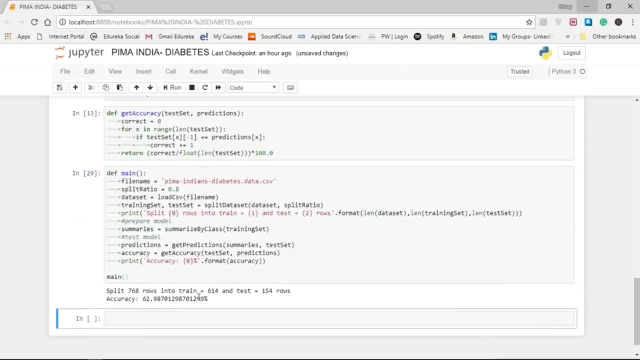 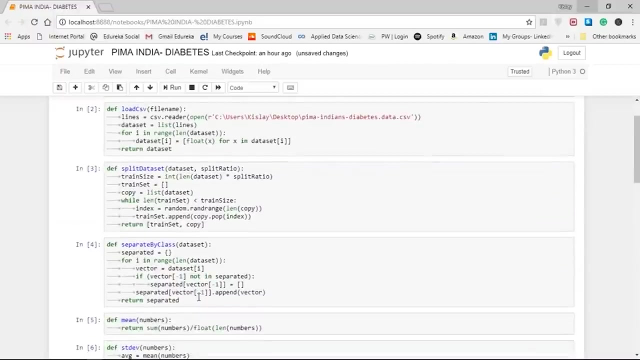 So, as you can see, we get the accuracy of 62%. so splitting it into 0.67 gave us a better result, which was 68%. so this is how you can implement a naive bias caution classifier. These are the step-by-step methods which you need to do in case of 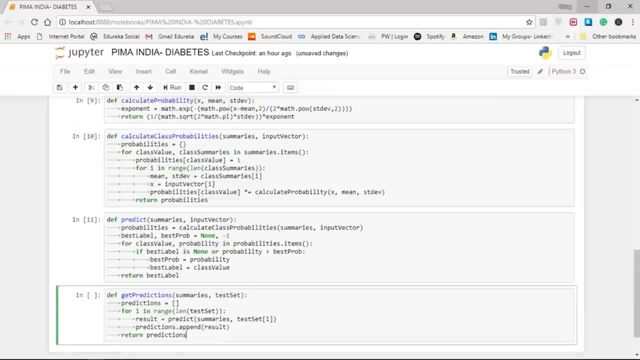 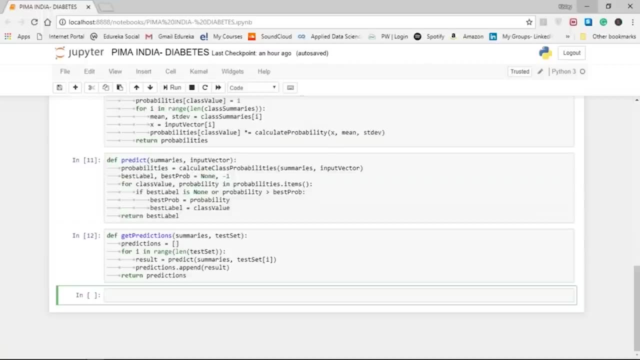 for that we use the get predictions method. now this method is used to calculate the predictions based upon the test data sets and the summary of the training data set. now the predictions can be compared to the class values in our test data set and classification accuracy can be. 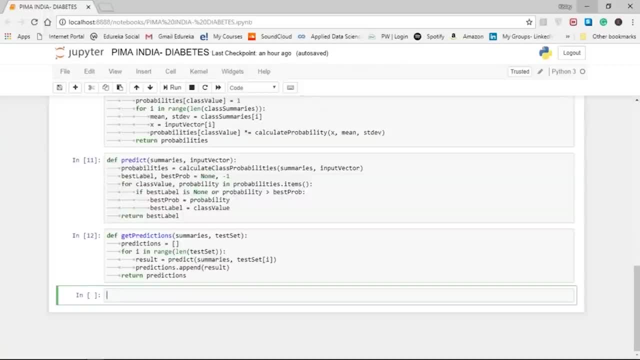 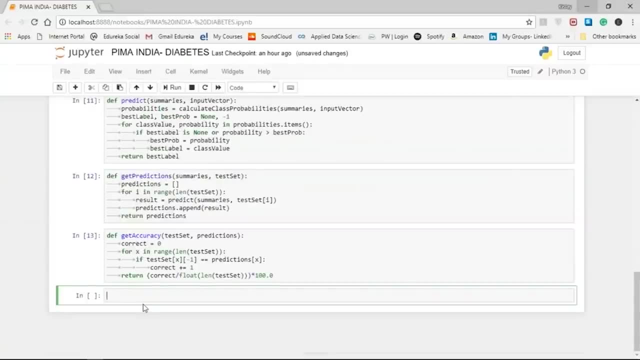 calculated as an accuracy ratio between the zeros and the hundred percent. now, the get accuracy method will calculate this accuracy ratio. Now, finally, to sum it all up, we define our main function. we call all these methods which we have defined earlier, one by one, to get the accuracy. 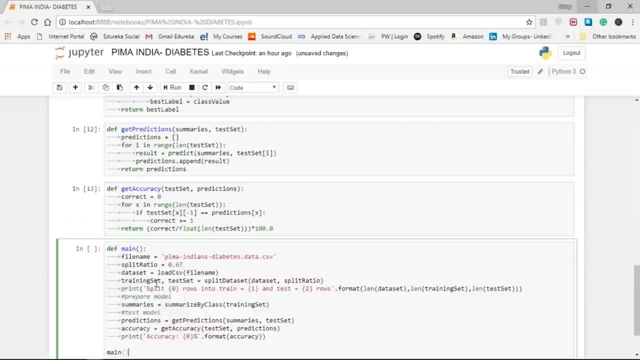 of the model which we have created. So, as you can see, this is our main function, in which we have the file name, We have to define the split ratio, We have the data set, We have the training and test data set. We are using the split data set method. next, 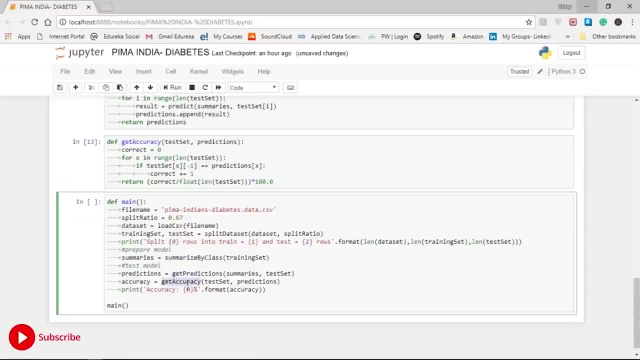 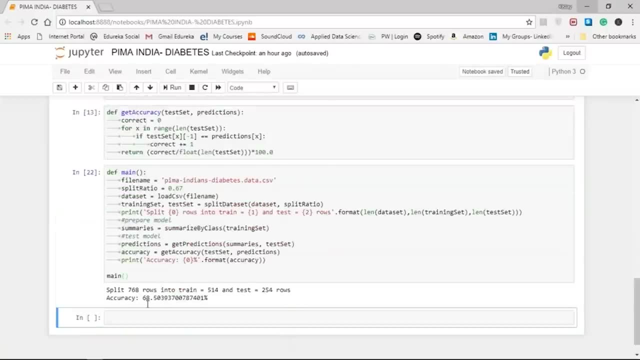 We are using the summarized by class function. We are using the get prediction and the get accuracy method as well. So, guys, as you can see, the output of this one gives us that we are splitting the 768 rows into 514, which is the training, and 254,. 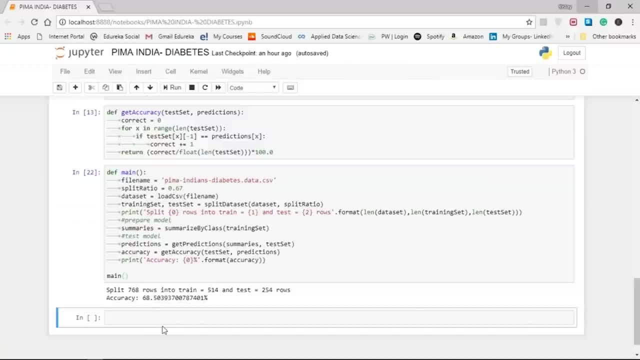 which is the test data set rows, and the accuracy of this model is 68%. now we can play with the amount of training and test data sets which are to be used here, So we can change the split ratio to 70s, to 38 days to 20. 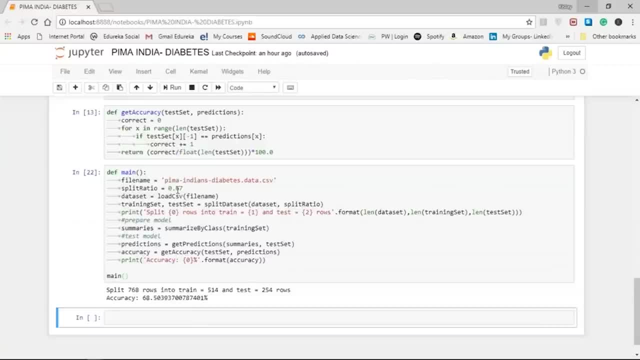 to get different sort of accuracy. So suppose I change the split ratio from 0.67 to 0.8.. So, as you can see, we get the accuracy of 62%. so splitting it into 0.67 gave us a better result, which was 68%. 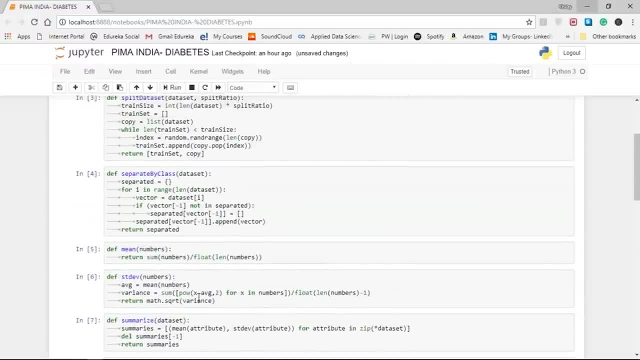 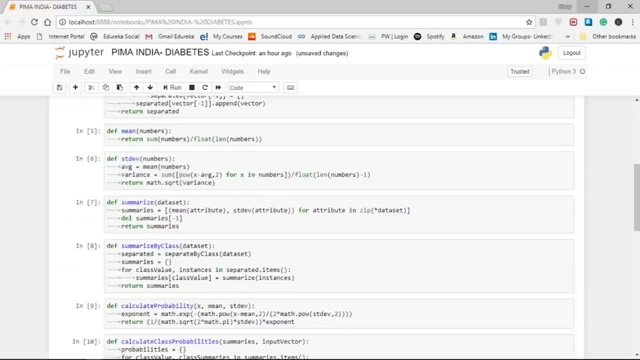 so this is how you can implement a naive bias caution classifier. These are the step-by-step methods which you need to do in case of using the naive bias classifier, but don't worry, We do not need to write all this many lines of code to make. 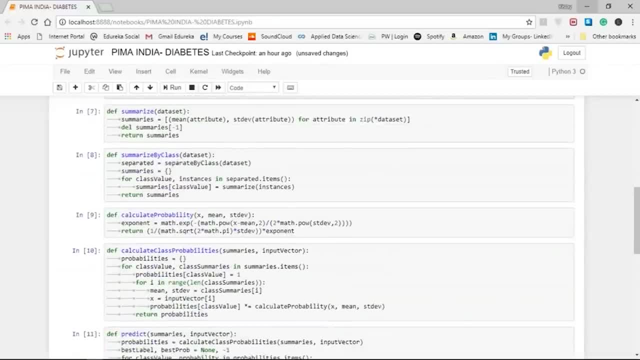 using the naive bias classifier. But don't worry, We do not need to write all this many lines of code to make a model. this way, the scikit-learn library comes into picture. the scikit-learn library has a predefined method or, as say, a predefined function of. 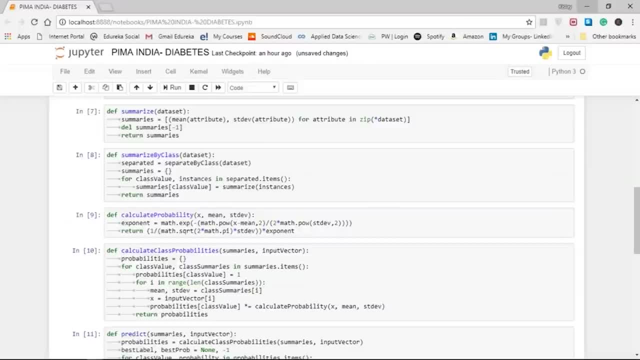 a model. this way, the scikit-learn library comes and into picture. the scikit-learn library has a predefined method or, as say, a predefined function of naive bias, which converts all of these lines of course, into merely just two or three lines of codes. 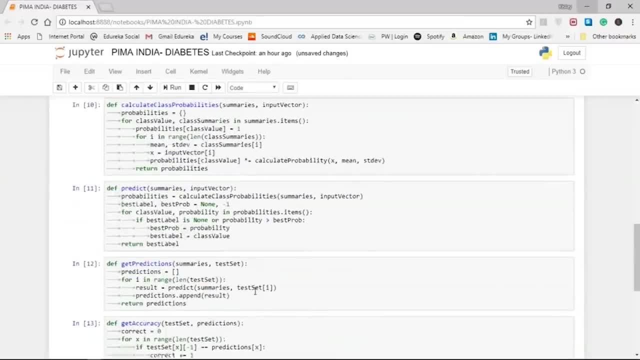 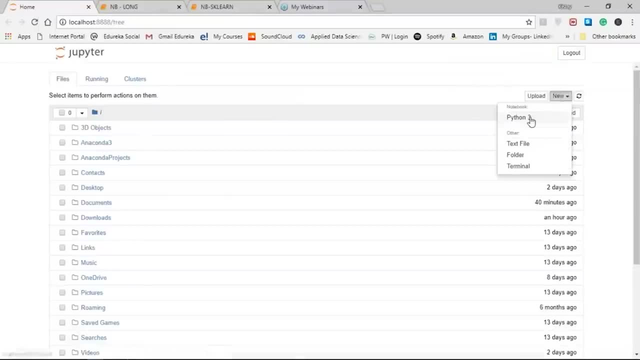 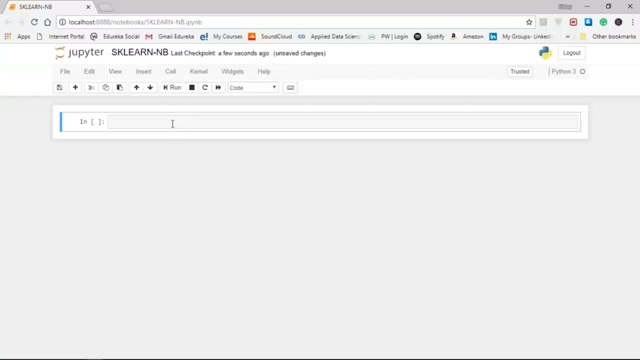 naive bias which converts all of these lines, of course, into merely just two or three lines of codes. So let me just open another Jupiter notebook, So let me name it as sklearn naive bias. Now, here we are going to use the most famous data set, which is the 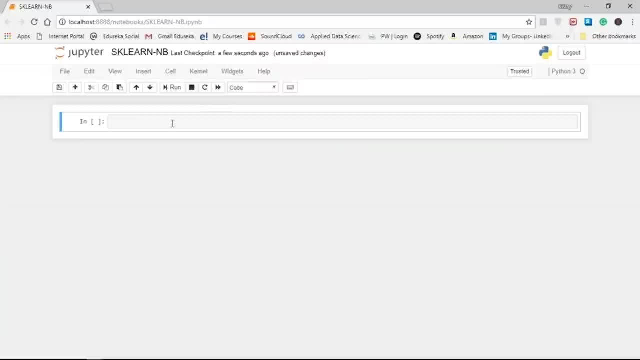 iris data set, now the iris flower data set, is a multivariate data set introduced by the British statistician and biologist Roland Fisher and based on this Fisher's linear discriminant model. This data set became a typical test case for many statistical classification techniques in machine learning. 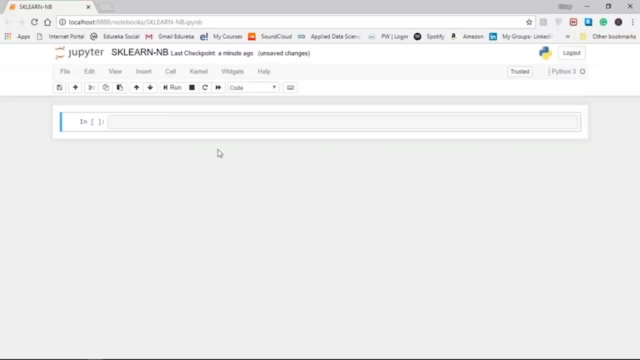 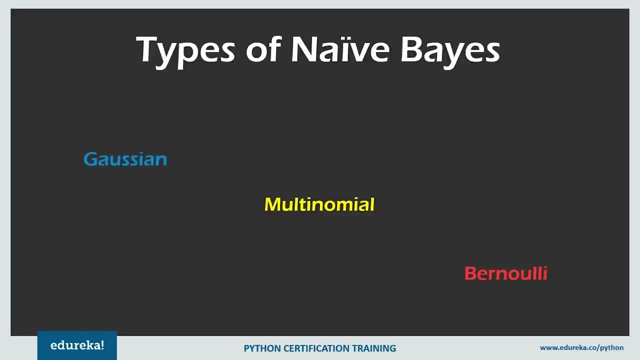 So here we are going to use the Gaussian NB model, which is already available in the sklearn. as I mentioned earlier, There were three types of naive bias, which are the Gaussian multinomial and the Bernoulli. So here we are going to use the Gaussian NB model, which is already. 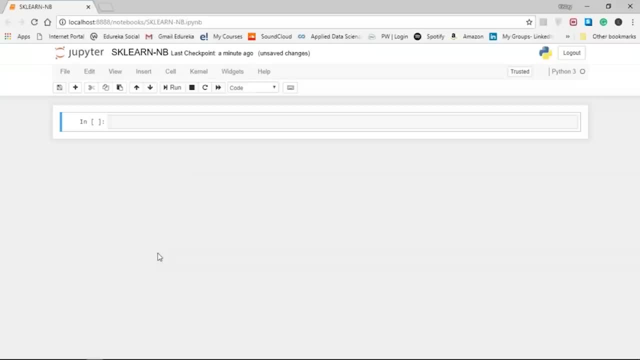 present in the sklearn library, which is the scikit-learn library. So, first of all, what we need to do is import the sklearn data sets and the metrics, and we also need to import the Gaussian NB. Now, once all these libraries are loaded, we need to load the data set. 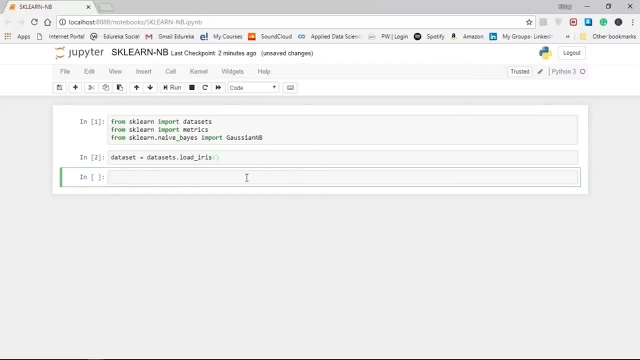 which is the iris data set. The next, what we need to do is fit a naive bias model to this data set. So, as you can see, we have so easily defined the model, which is the Gaussian NB, which contains all the programming which I just showed you earlier, all the methods which are taking the 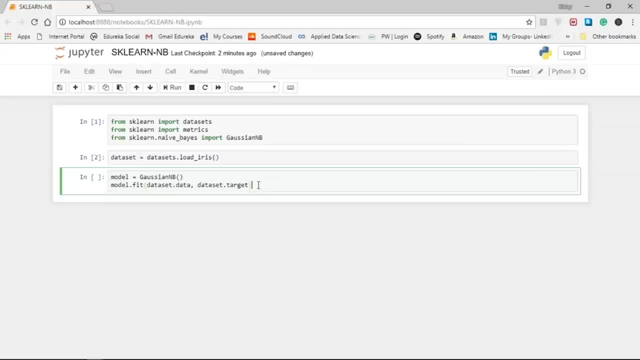 input, calculating the mean, the standard deviation, separating it by class and, finally, making predictions and calculating the prediction accuracy. All of these comes under the Gaussian NB method, which is inside, Already present in the sklearn library. We just need to fit it according to the data set which we have. 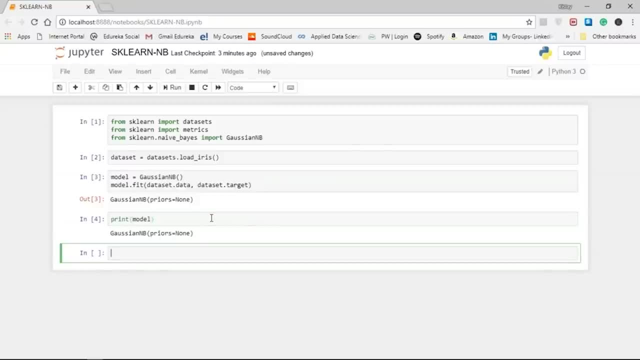 here. So next, if we print the model we see, which is the Gaussian NB model, the next what we need to do is make the predictions. So the expected output is data set, dot target and the predicted is using the predicted model. and the model we are using is the. 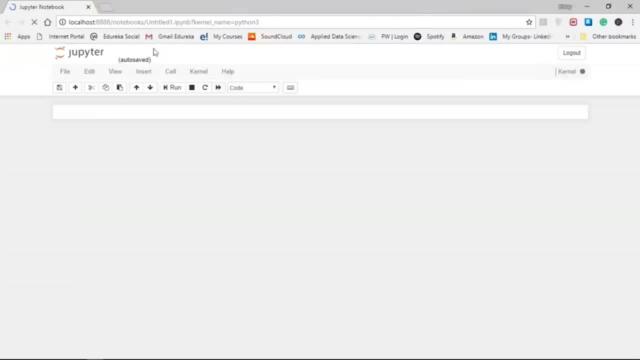 So let me just open another Jupiter notebook, So let me name it as sklearn naive bias. Now here we are going to use the most famous data set, which is the iris data set. now the iris flower data set is a multivariate data set introduced. 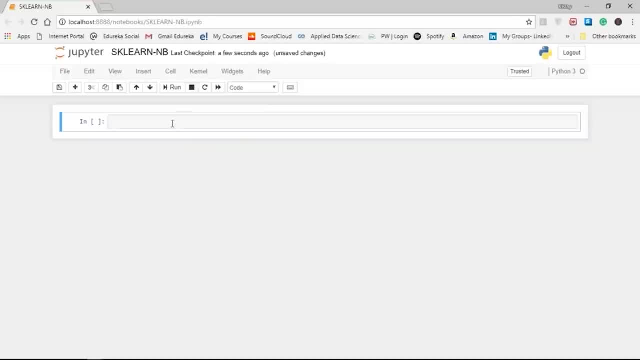 by the British statistician and biologist Roland Fisher, and based on this Fisher's linear discriminant model, This data set became a typical test case for many statistical classification techniques in machine learning. So here we are going to use the Gaussian NB model, which is already available in the sklearn. 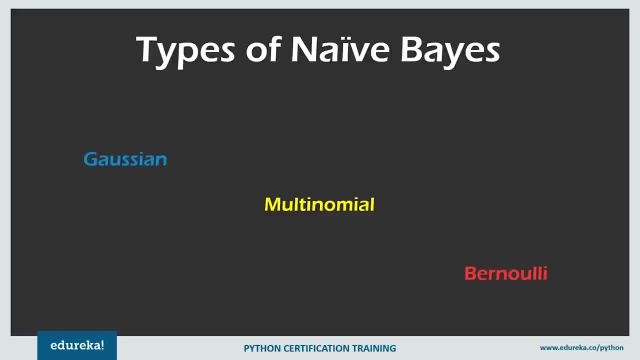 As I mentioned earlier, there were three types of naive bias, which are the Gaussian multinomial and the Bernoulli. So here we are going to use the Gaussian NB model, which is already present in the sklearn library, which is the cycle and library. 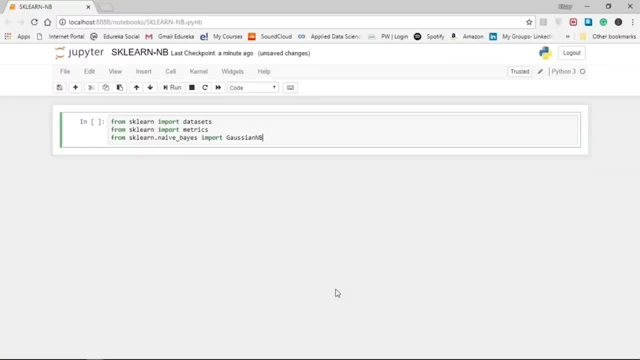 So, first of all, what we need to do is import the sklearn data sets and the metrics, and we also need to import the Gaussian NB. Now, once all these libraries are loaded, we need to load the data set, which is the iris data set. 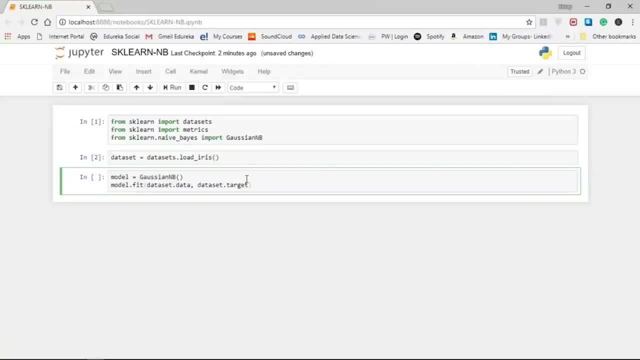 The next. what we need to do is fit a naive bias model to this data set. So, as you can see, we have so easily defined the model, which is the Gaussian NB, which contains all the programming which I just showed you earlier. 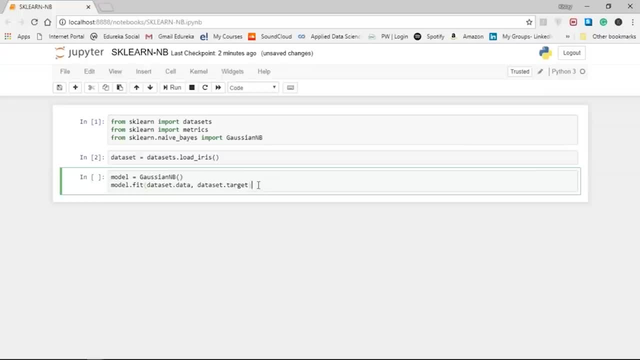 All the methods which are taking the input, calculating the mean, the standard deviation, separating it by class, Then, finally, making predictions and calculating the prediction accuracy. all of these comes under the Gaussian NB method, which is inside, already present in the sklearn library. We just need to fit it according to the data set. 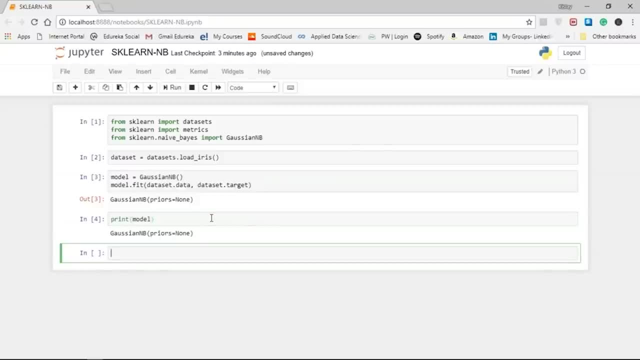 which we have here. So next, if we print the model we see, which is the Gaussian NB model, The next what we need to do is make the predictions. So the expected output is data set, dot target and the predicted is using the predicted model. and the model we are using is 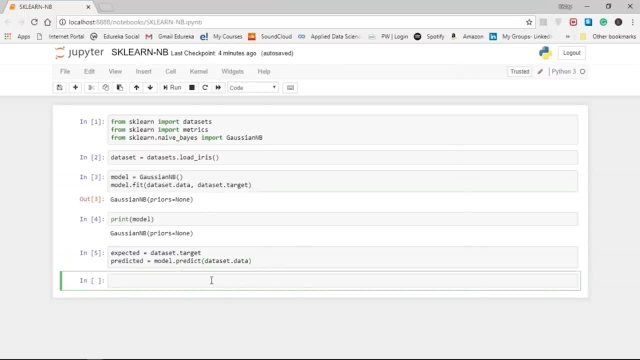 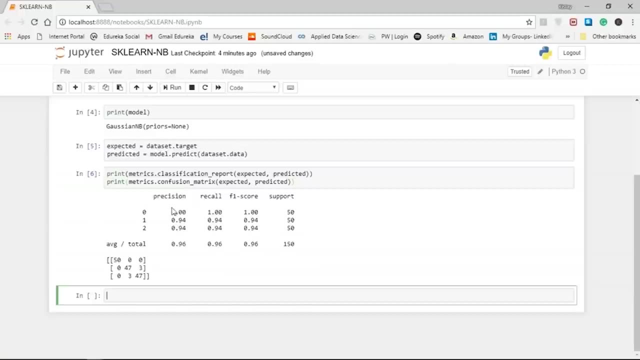 the Gaussian NB here. Now to summarize the model which is created. we calculate the confusion matrix and the classification report. So, guys, as you see the classification report, we have the precision of 0.90.. 6. We have the recall of 0.96. 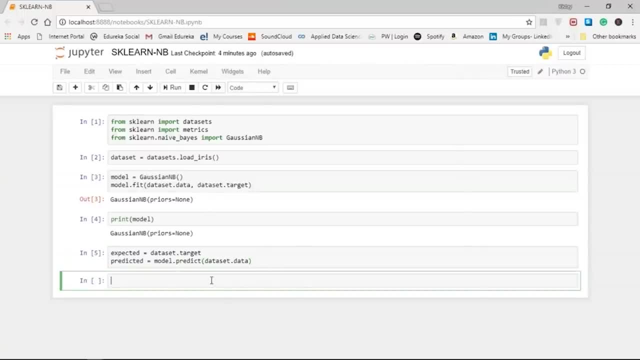 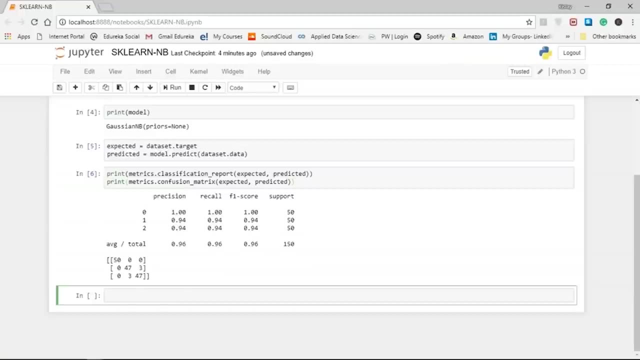 Gaussian NB here. Now to summarize the model which is created. we calculate the confusion Matrix and The classification report. So, guys, as you see the classification report, we have the precision of 0.96.. We have the recall of 0.96. 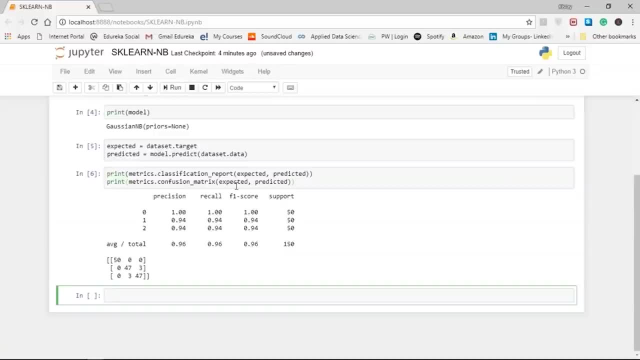 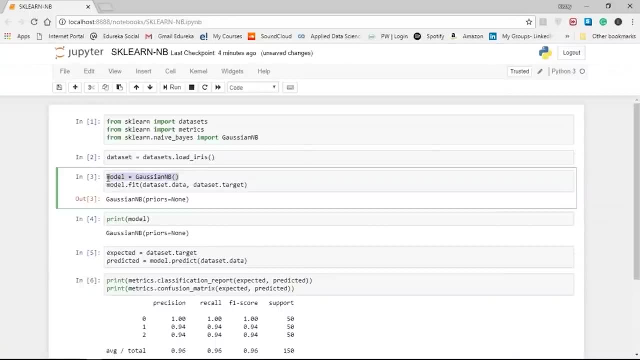 We have the F1 score and the support and, finally, if you print our confusion Matrix, as you can see, it gives us this output. So, as you can see, using the Gaussian NB method, just putting it in the model and using any of the data set fitting the model, 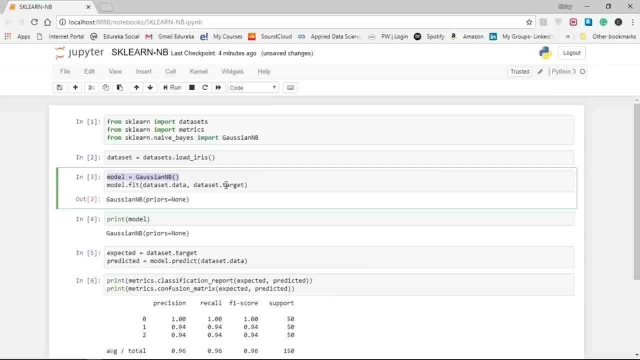 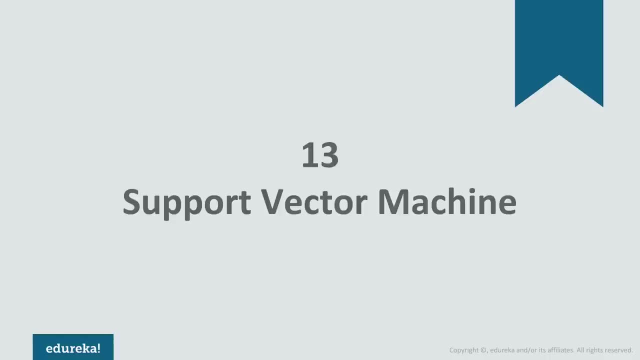 which you created into a particular data set, and getting the desired output Is so easy with the scikit-learn library. SVM, or support vector machine, is one of the most effective machine learning classifier, and it has been used in various fields such as face recognition, cancer classification and so on. today's 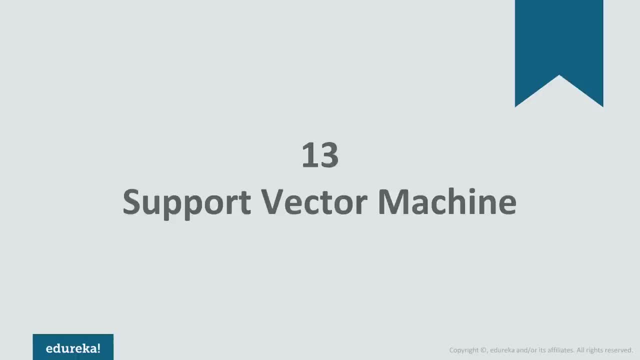 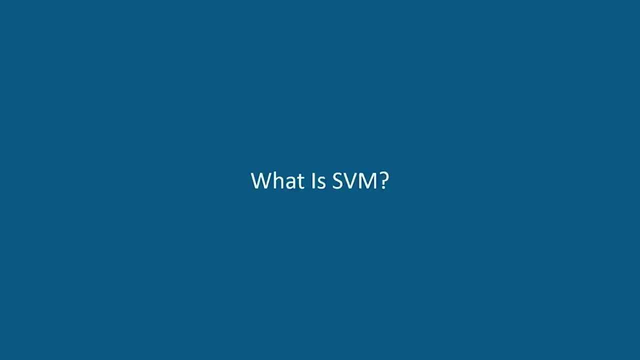 session is dedicated to how SVM works, the various features of SVM and how it is used in the real world. All right, Okay, Now let's move on and see what SVM algorithm is all about. So, guys, SVM, or support vector machine, is a supervised learning. 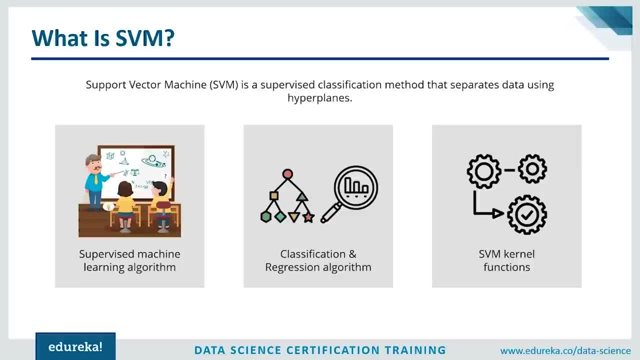 algorithm which is mainly used to classify data into different classes. Now, unlike most algorithms, SVM makes use of a hyperplane which acts like a decision boundary between the various classes. in general, SVM can be used to generate multiple separating hyperplanes so that the data is divided into segments. 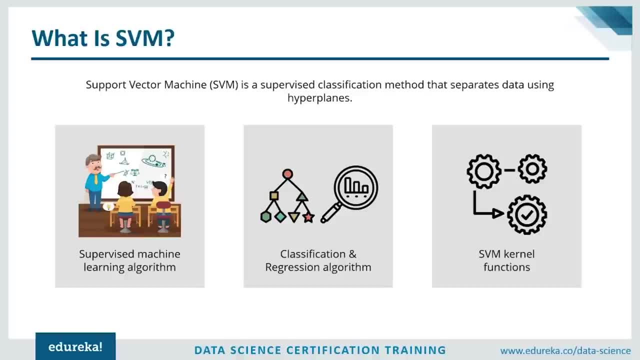 Okay, and each of these segments will contain only one kind of data. It's mainly used for classification purpose, wherein you want to classify a data into two different segments depending on the features of the data. now, before moving any further, Let's discuss a few features of SVM. 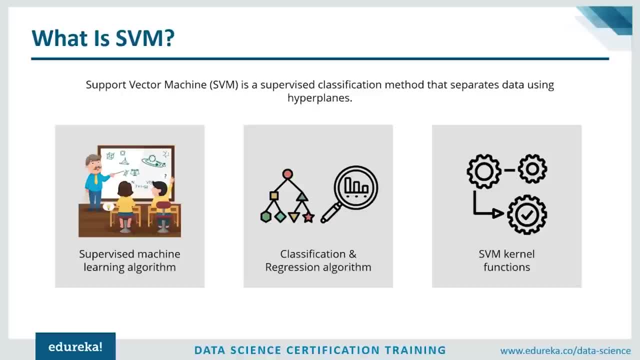 Like I mentioned earlier, SVM is a supervised learning algorithm. This means that SVM trains on a set of label data. SVM studies the label training data and then classifies any new input data depending on what it learned in the training phase. a main advantage of support vector machine. 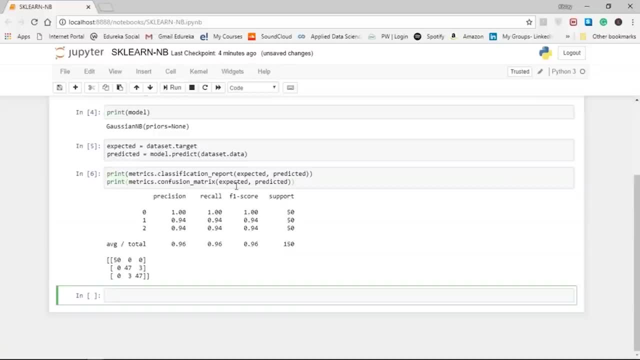 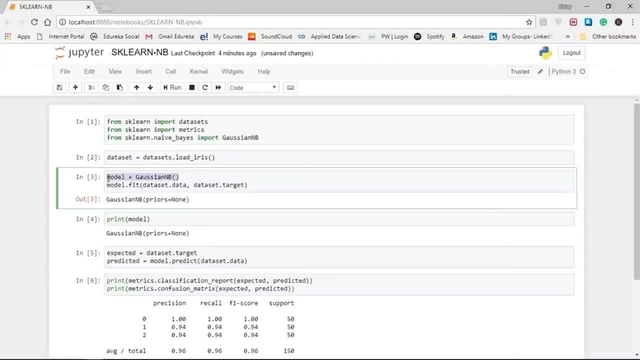 We have the F1 score and the support and, finally, if you print our confusion Matrix, as you can see, it gives us this output. So, as you can see, using the Gaussian NB method, just putting it in the model and using any of the data set fitting the 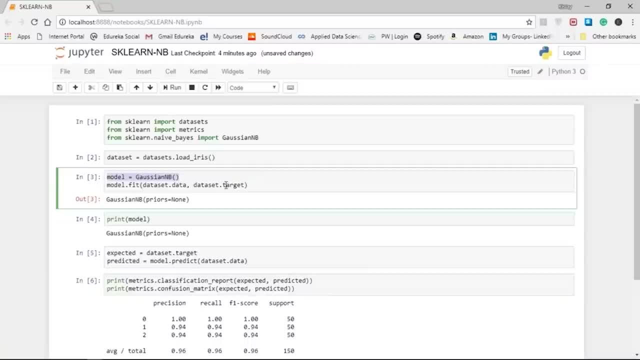 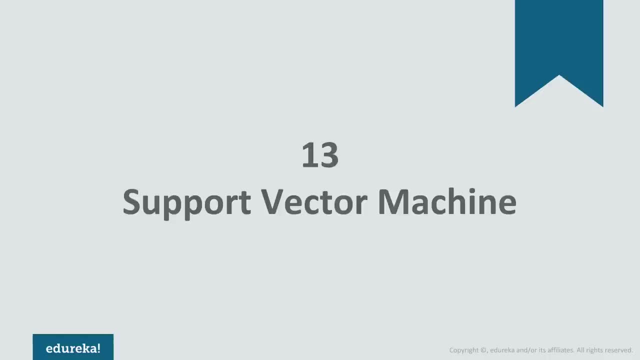 model which you created into a particular data set, and getting the desired output is so easy with the scikit-learn library. SVM, or support vector machine, is one of the most effective machine learning classifier and it has been used in various fields such as face recognition. 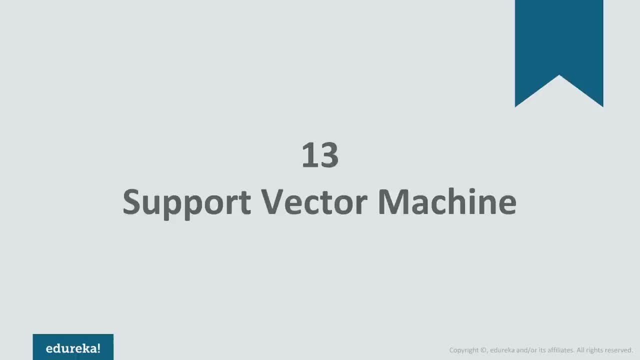 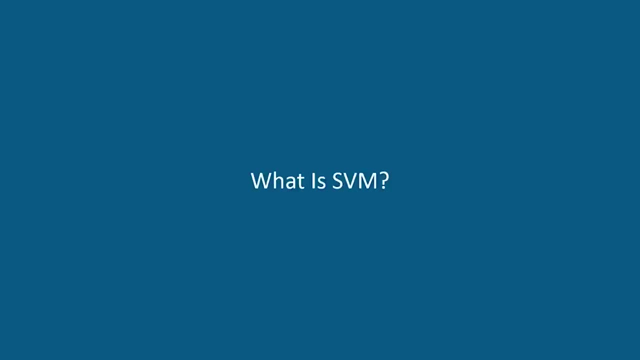 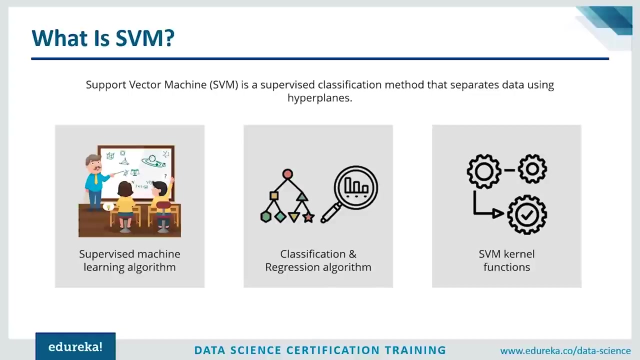 cancer classification and so on. Today's session is dedicated to how SVM works, the various features of SVM and how it is used in the real world. All right, Okay, Now let's move on and see what SVM algorithm is all about. So, guys, SVM or support vector machine, is a supervised learning 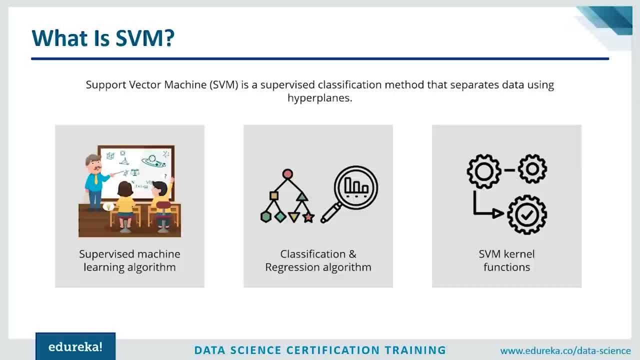 algorithm which is mainly- mainly- used to classify data into different classes. Now, unlike most algorithms, SVM makes use of a hyperplane which acts like a decision boundary between the various classes. in general, SVM can be used to generate multiple separating hyperplanes so that the data is divided into segments. 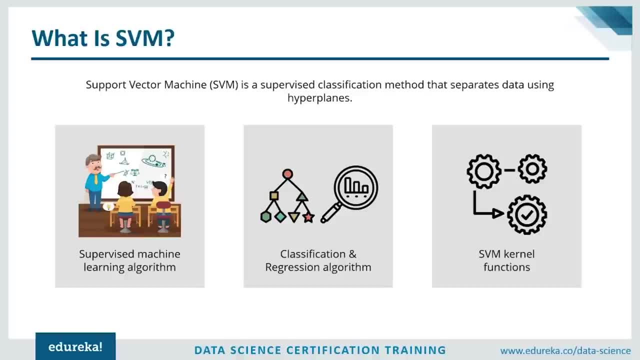 Okay, and each of these segments will contain only one kind of data. It's mainly used for classification purpose, wherein you want to classify a data into two different segments, depending on the feature: The data. now, before moving any further, Let's discuss a few features of SVM. 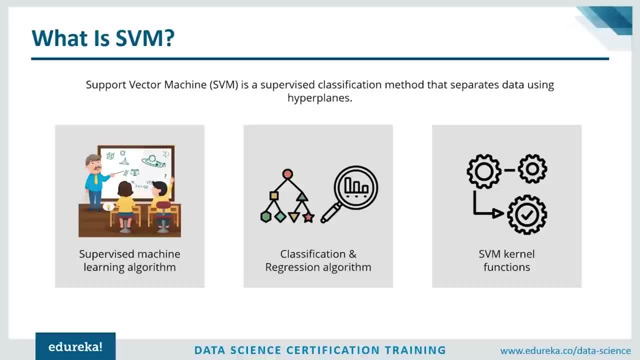 Like I mentioned earlier, SVM is a supervised learning algorithm. This means that SVM trains on a set of label data. SVM studies the label training data and then classifies any new input data depending on what it learned in the training phase. a main advantage of support vector machine is that it can be used for both classification and 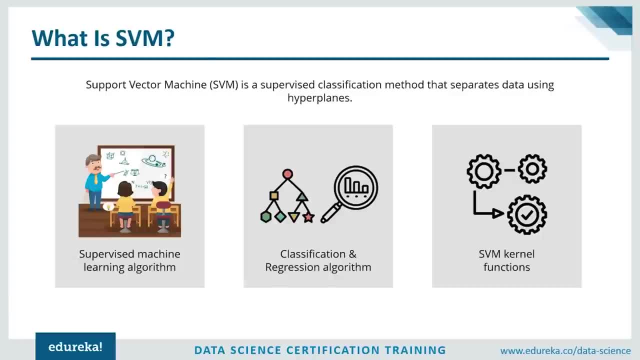 regression problems. All right. now, even though SVM is mainly known for classification, the SVR, which is the support vector, regressor, is used for regression problems. All right, so SVM can be used both for classification and for regression. Now, This is one of the reasons why a lot of people prefer SVM, because 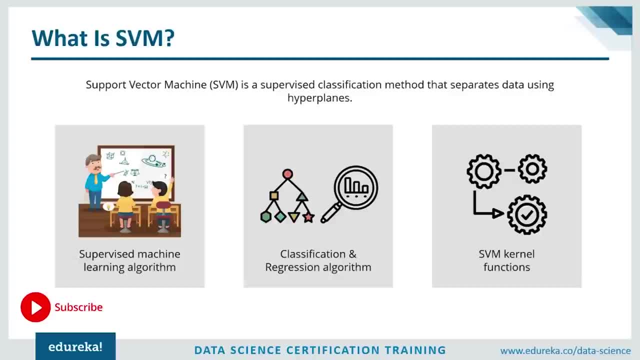 Is that it can be used for both classification and regression problems. All right. Now, even though SVM is mainly known for classification, the SVR, which is the support vector, regressor, is used for regression problems. All right, So SVM can be used both for classification and for regression. 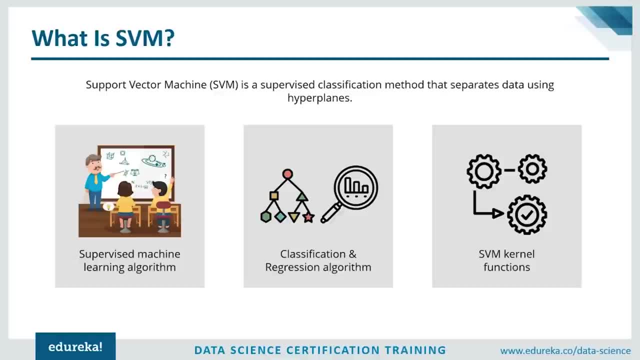 Now, this is one of the reasons why a lot of people prefer SVM: because it's a very good classifier and, along with that, it is also used for regression. Okay, Another feature is the SVM kernel Functions. SVM can be used for classifying nonlinear data by using: 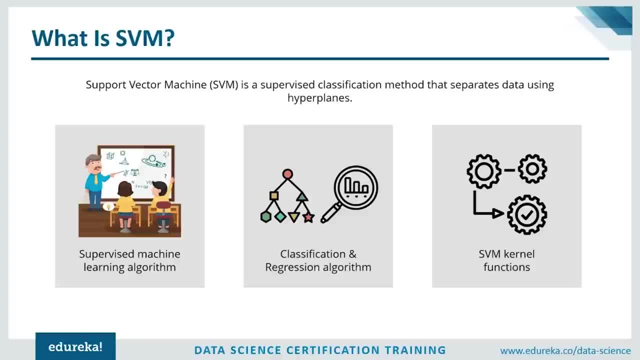 the kernel trick. the kernel trick basically means to transform your data into another dimension so that you can easily draw a hyper plane between the different classes of the data. All right, nonlinear data is basically data which cannot be separated with a straight line. All right. 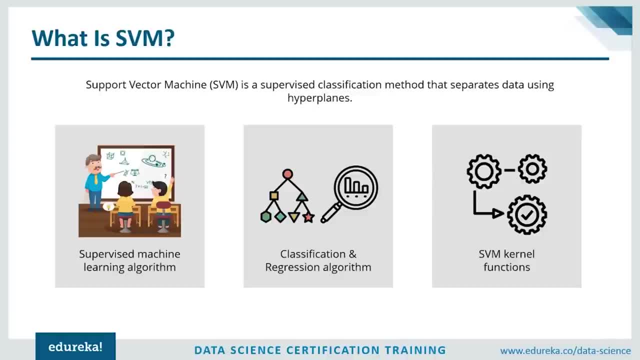 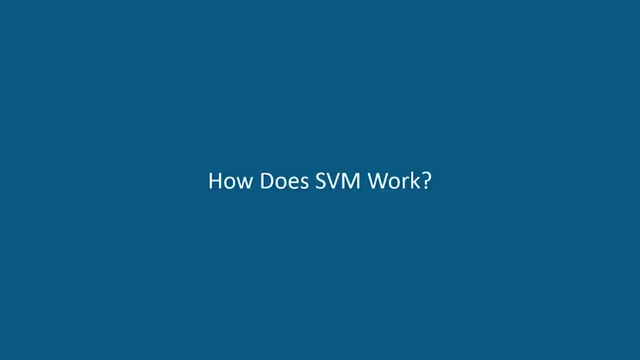 So SVM can even be used on nonlinear data sets. You just have to use a kernel functions to do this. All right, So, guys, I hope you all are clear with the basic concepts Of SVM. Now let's move on and look at how SVM works. 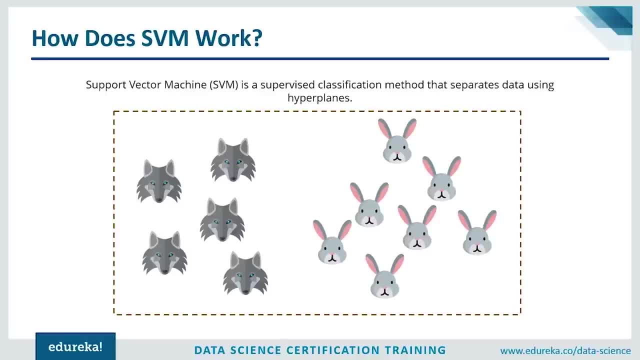 So there's an order to understand how SVM works. Let's consider a small scenario. Now for a second. pretend that you own a farm, Okay, And let's say that you have a problem and you want to set up a fence to protect your rabbits from the pack of wolves. 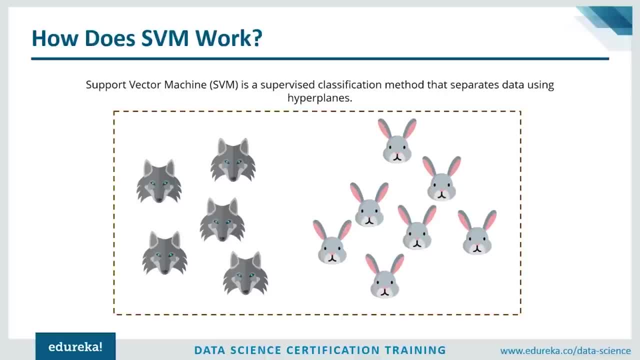 Okay, but where do you build your fence? one way to get around the problem is to build a classifier based on the position of the rabbits and wolves in your pasture. So what I'm telling you is you can classifier The group of rabbits as one group and draw a decision. boundary. 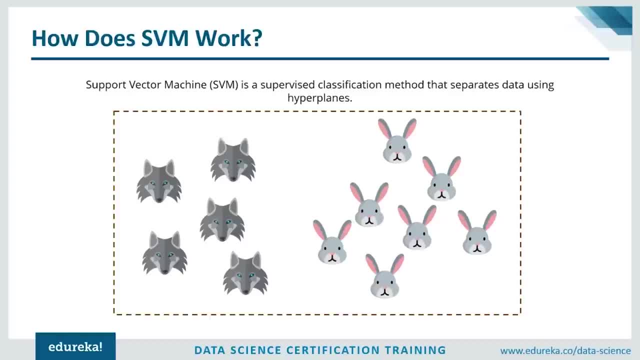 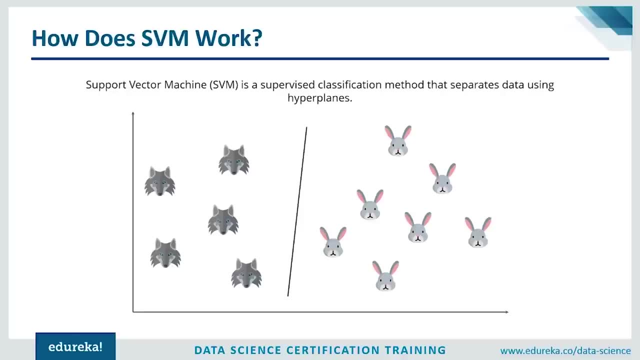 between the rabbits and the world. All right, So if I do that and if I try to draw a decision boundary between the rabbits and the wolves, it looks something like this: Okay, Now you can clearly build a fence along this line. in simple terms, 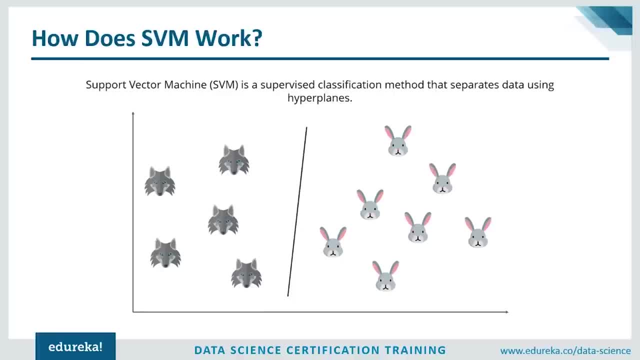 This is exactly how SVM work. It draws a decision boundary, which is a hyperplane, between any two classes in order to separate them or classify them. Now I know you're thinking: How do you know where to draw a hyperplane? The basic principle behind SVM is to draw a hyperplane that best. 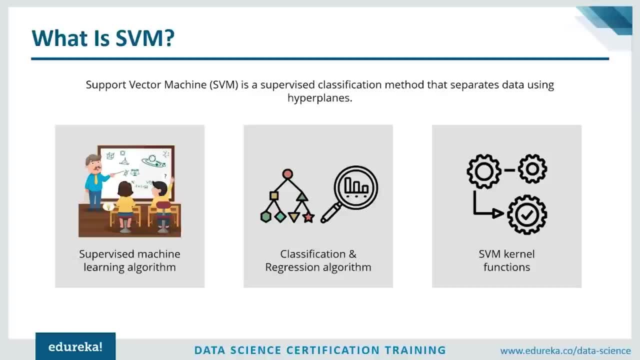 it's a very good classifier and along with that, it is also used for regression. Okay, another feature is the SVM kernel functions. SVM can be used for classifying nonlinear data by using the kernel trick. the kernel trick basically means to transform your data into another dimension. 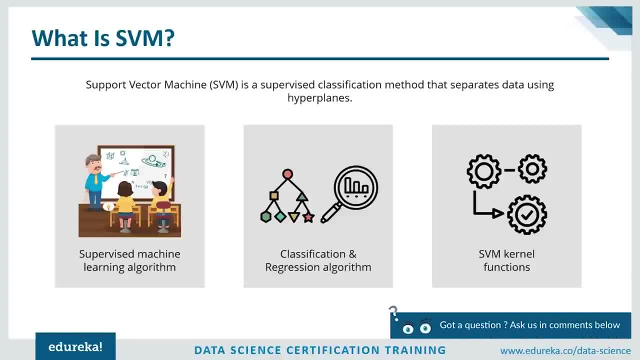 so that you can easily draw a hyperplane between the different classes of the data. All right. nonlinear data is basically data which cannot be separated with a straight line. All right, so SVM can even be used on nonlinear data sets. You just have to use a kernel functions to do this. 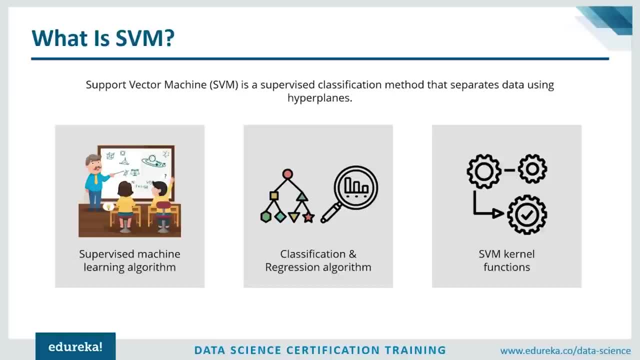 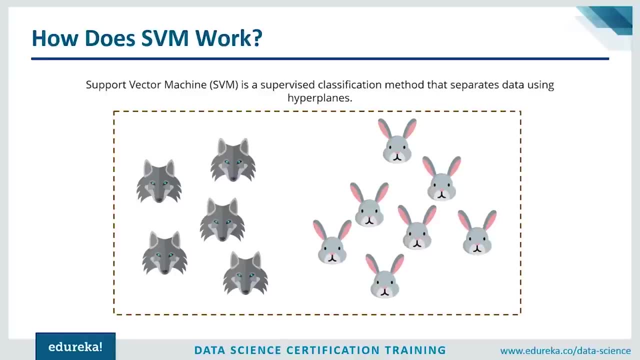 All right. So, guys, I hope you all are clear with the basic concepts of SVM. Now let's move on and look at how SVM works. So, guys, in order to understand how SVM works, Let's consider a small scenario. Now for a second. pretend that you own a farm. 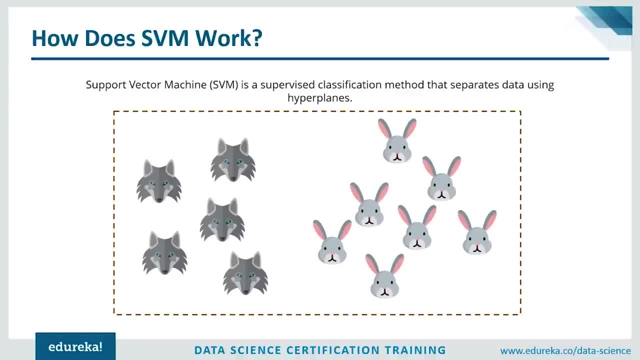 Okay, and let's say that you have a problem and you want to set up a fence to protect your rabbits from the pack of wolves. Okay, but where do you build your fence? One way to get around the problem is to build a classifier based. 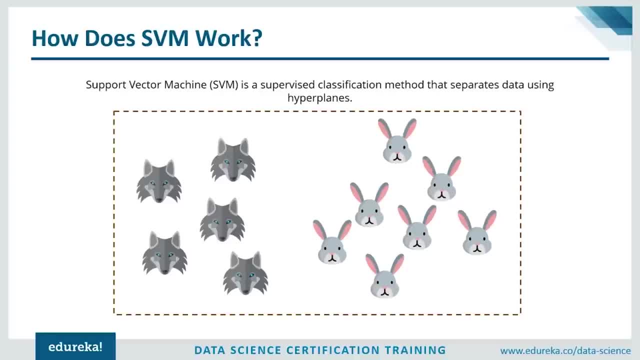 on the position of the rabbits and wolves in your pasture. So what I'm telling you is you can classify the group of rabbits as one group and draw a decision boundary between the rabbits and the wolves, All right. So if I do that and if I try to draw a decision boundary between 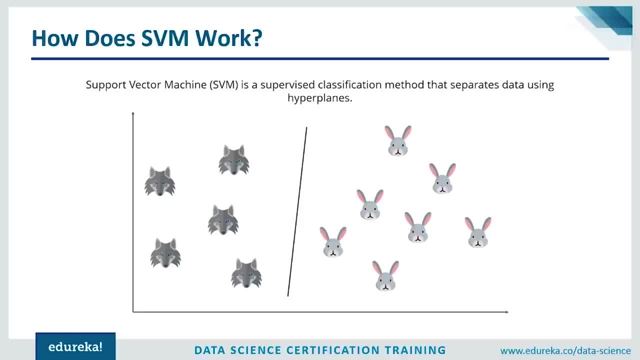 the rabbits and the wolves. it looks something like this: Okay, Now you can clearly build a fence along this line. in simple terms, This is exactly how SVM work. It draws a decision boundary, which is a hyperplane between any two classes, in order to separate them or classify them. 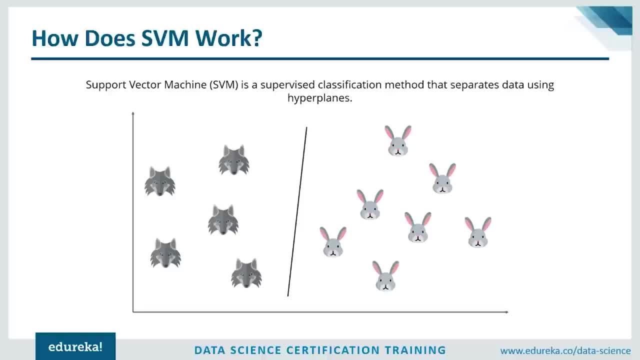 Now I know you're thinking: how do you know where to draw a hyperplane? The basic principle behind SVM is to draw a hyperplane that best separates the two classes. In our case, the two classes are the rabbits and the wolves. So you start off by drawing a random hyperplane and then you 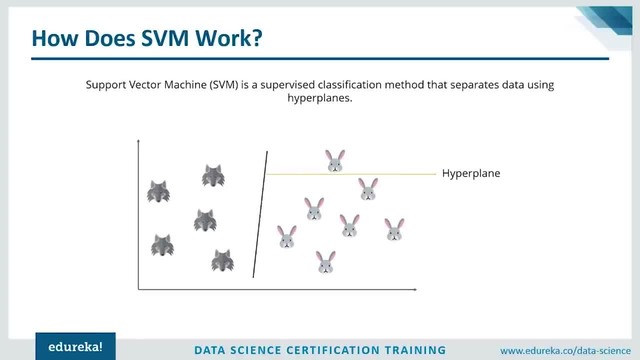 check the distance between the hyperplane and the closest data points from each class. These closest or nearest data points to the hyperplane are known as support vectors, and that's where the name comes from: support vector machine. So, basically, the hyperplane is drawn based on these support vectors. 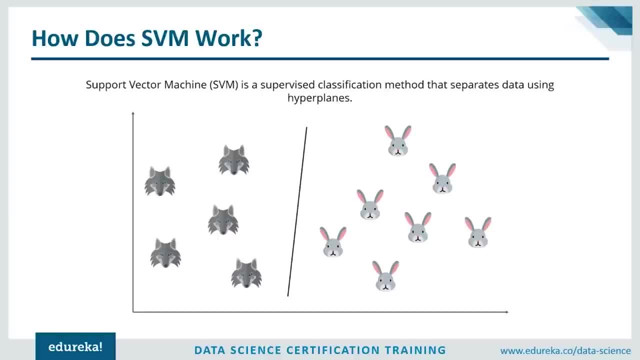 separates the two classes. In our case, the two classes are the rabbits and the wolves. So you start off by drawing a random hyperplane and then you check the distance between the hyperplane and the closest data points from each class. These closest or nearest data points to the hyperplane are known as. 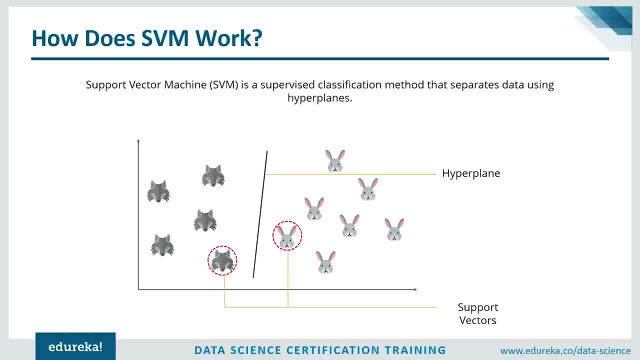 support vectors, And that's where the name comes from: support vector machine. So basically, a hyperplane is drawn based on these support vectors. So, guys, an optimum hyperplane will have a maximum distance from each of these support vectors. Alright, so basically, the hyperplane which has the maximum distance. 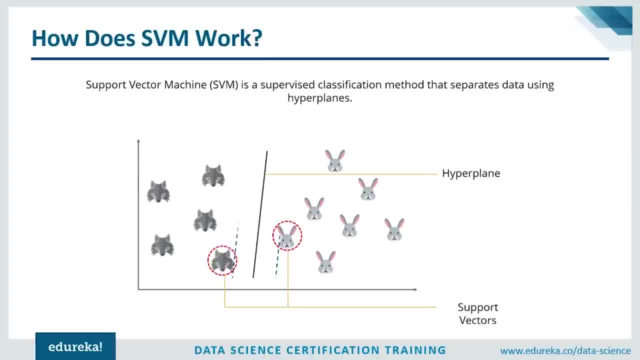 from the support vectors is the most optimum hyperplane, and this distance between the hyperplane and the support vectors is known as the margin Alright. so to sum it up, SVM is used to classify data by using a hyperplane, such that the distance between the hyperplane and the support 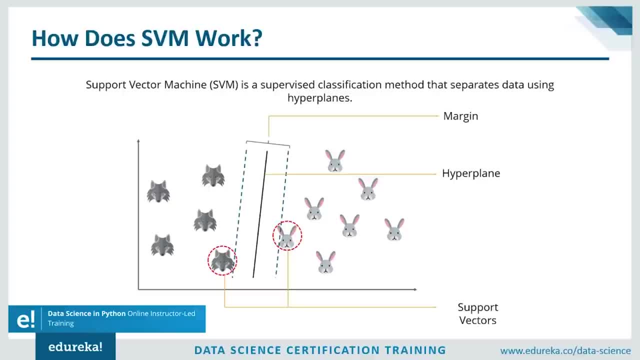 vectors is maximum. So basically, your margin has to be maximum. All right, that way you know that you're actually separating your classes. All right, because the distance between the two classes is maximum. Okay, Now let's try to solve a problem. 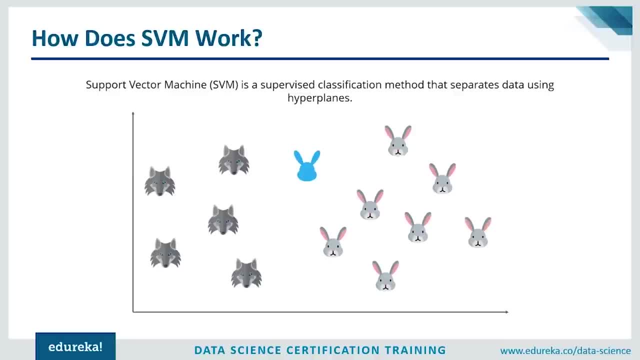 Okay. So let's say that I input a new data point. Okay, This is the new data point, and now I want to draw a hyperplane such that it best separates the two classes. Okay, so I start off by drawing a hyperplane like this, and then I 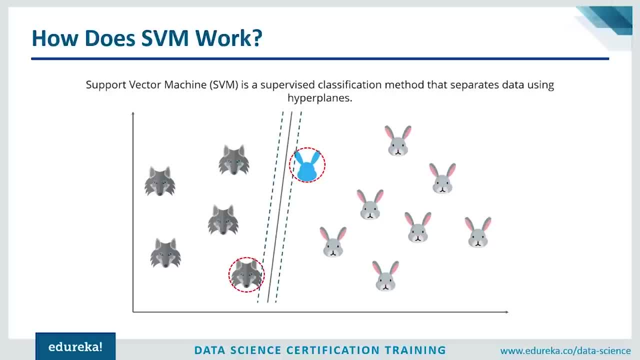 check the distance between the hyperplane and the support vectors. Okay, so I'm trying to check if the margin is maximum for this hyperplane. But what if I draw a hyperplane which is like this: All right, Now I'm going to check the support vectors over here. 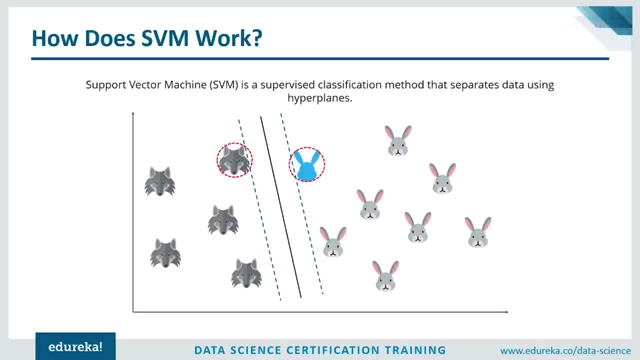 Then I'm going to check the distance from the support vectors and for this hyperplane It's clear that the margin is more Alright. when you compare the margin of the previous one to this hyperplane, it is more So. the reason why I'm choosing this hyperplane is because the 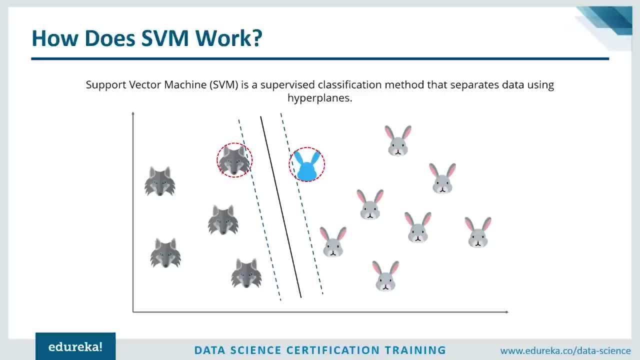 distance between the support vectors and the hyperplane is maximum in this scenario. Okay so, guys, this is how you choose a hyperplane. You basically have to make sure that the hyperplane has a maximum margin. All right, it has to best separate the two classes. 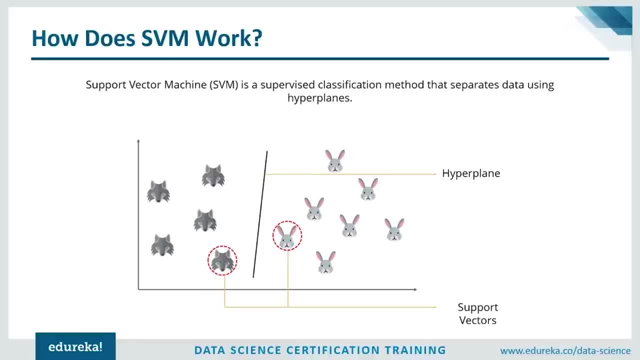 So, guys, an optimum hyperplane will have a maximum distance for the hyperplane Since from each of these support vectors. All right. So basically, the hyperplane which has the maximum distance from the support vectors is the most optimum hyperplane, and this distance between 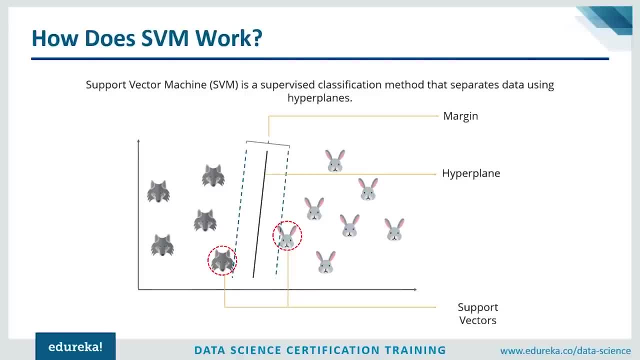 the hyperplane and the support vectors is known as the margin. All right, So to sum it up, SVM is used to classify data by using a hyperplane, such that the distance between the hyperplane and the support vectors is maximum. So basically, your margin has to be maximum. 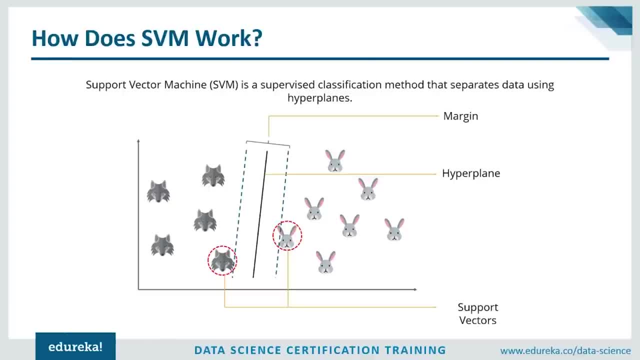 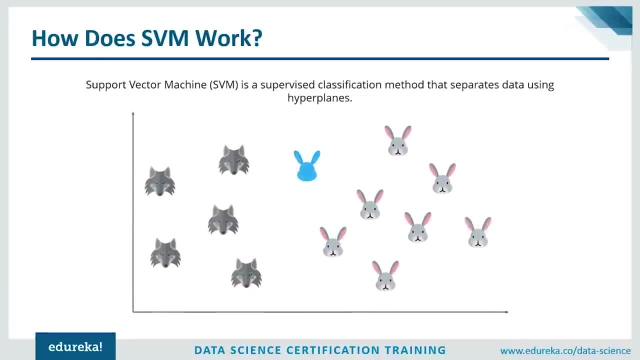 All right, that way you know that you're actually separating your classes. All right, because the distance between the two classes is maximum. Okay, Now let's try to solve a problem. Okay, So let's say that I input a new data point. 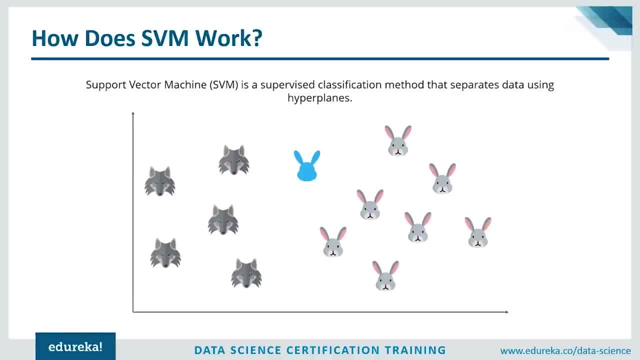 Okay, This is the new data point, and now I want to draw a hyperplane such that it best separates the two classes. Okay, so I start off by drawing a hyperplane like this, and then I check the distance between the hyperplane and the support vectors. 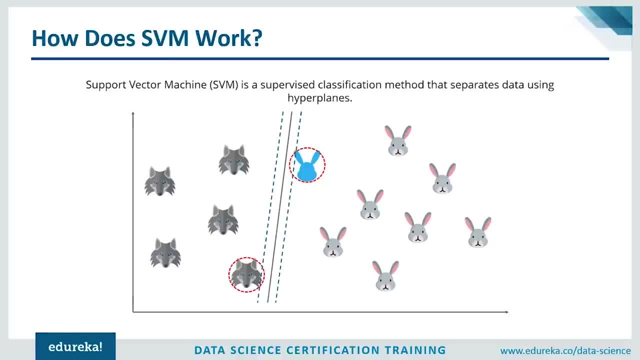 Okay, so I'm trying to check if the margin is maximum for this hyperplane. But what if I draw a hyperplane Which is like this: All right, Now I'm going to check the support vectors over here, Then I'm going to check the distance from the support vectors and 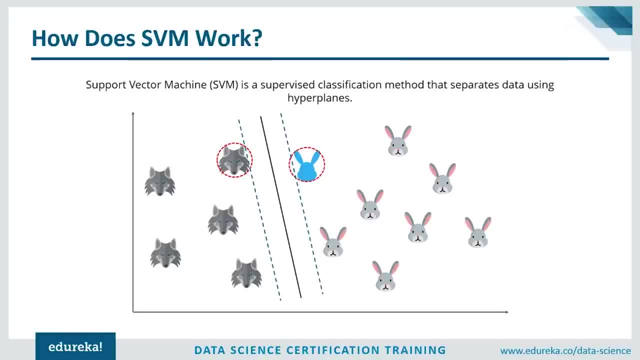 for this hyperplane, It's clear that the margin is more All right. when you compare the margin of the previous one to this hyperplane, it is more So. the reason why I'm choosing this hyperplane is because the distance between the support vectors and the hyperplane is maximum in this. 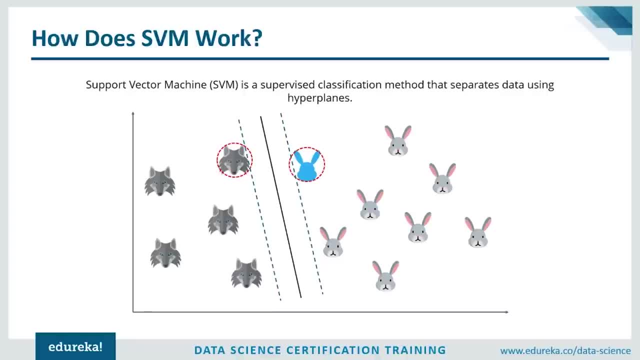 scenario: Okay. So guys, this is how you choose a hyperplane. You basically have to make sure that the hyperplane has a maximum margin. All right, it has to best separate the two classes, All right, Okay, So far it was quite easy. 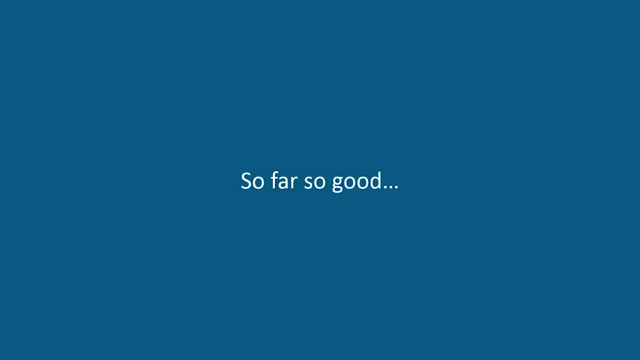 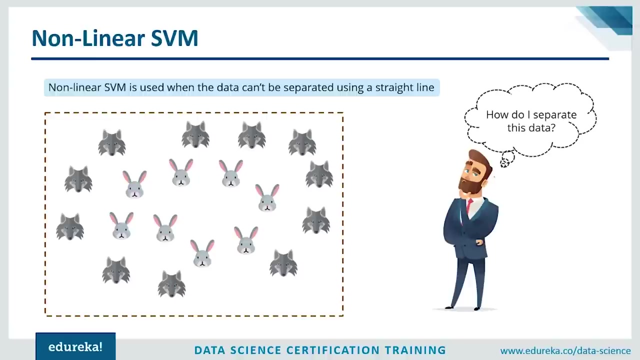 Our data was linearly separable, which means that you could draw a straight line to separate the two classes. All right, but what will you do if the data set is like this? You possibly can't draw a hyperplane like this. All right, it doesn't separate the two classes at all. 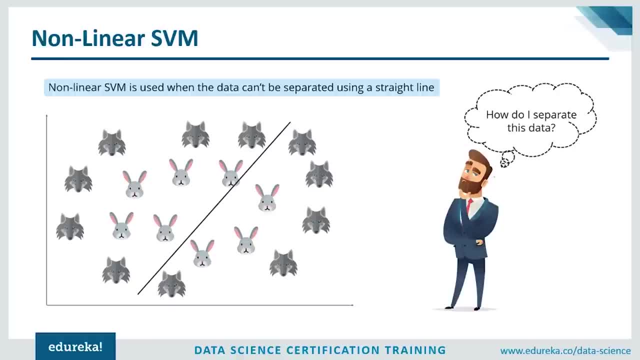 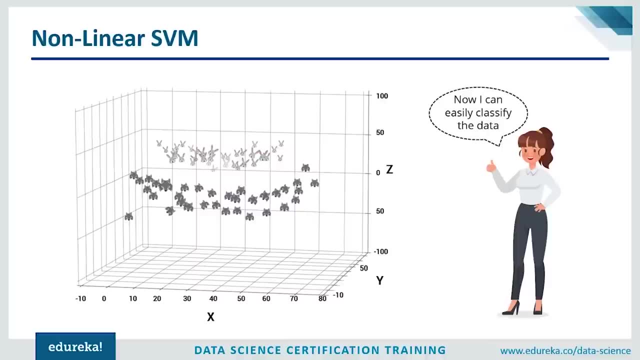 So what do you do in such situations? Now, earlier in the session I mentioned how a kernel can be used to transform data Into another dimension that has a clear dividing margin between the classes of data. All right, so kernel functions offer the user this option of transforming. 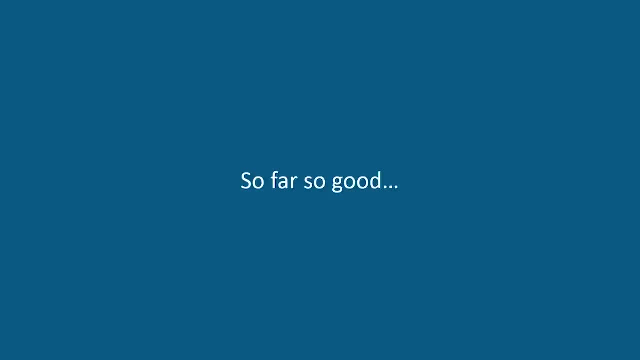 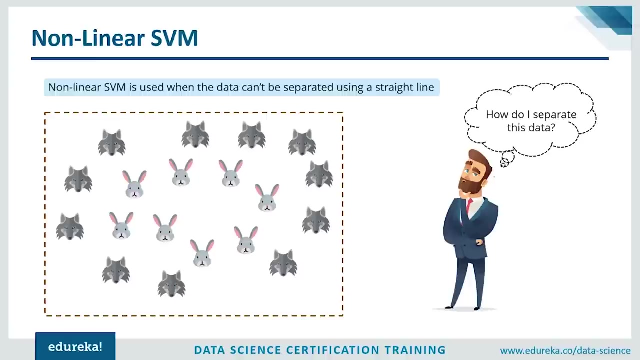 All right, Okay, So far it was quite easy. Our data was linearly separable, which means that you could draw a straight line to separate the two classes. All right, but what will you do if the data set is like this: 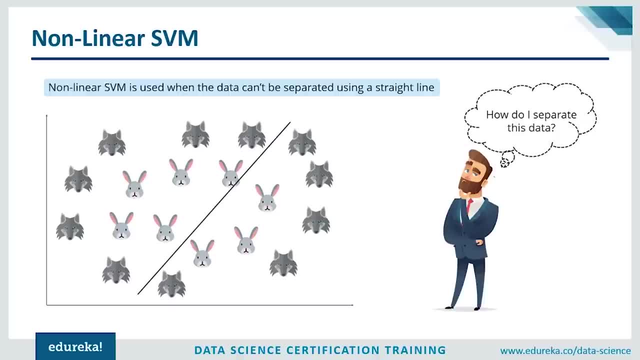 You possibly can't draw a hyperplane like this. All right, it doesn't separate the two classes at all. So what do you do You do in such situations Now, earlier in the session, I mentioned how a kernel can be used to. 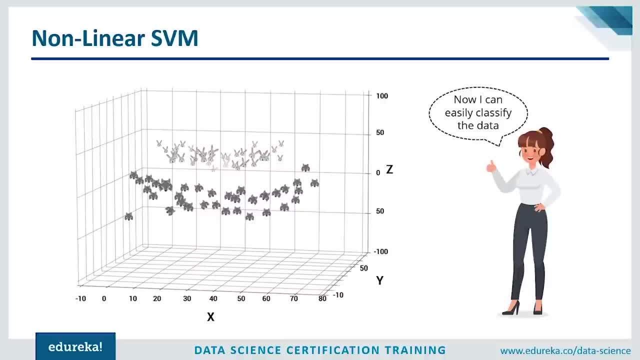 transform data into another dimension that has a clear dividing margin between the classes of data. All right. so kernel functions offer the user this option of transforming nonlinear spaces into linear ones. Nonlinear data set is the one that you can't separate using a straight. 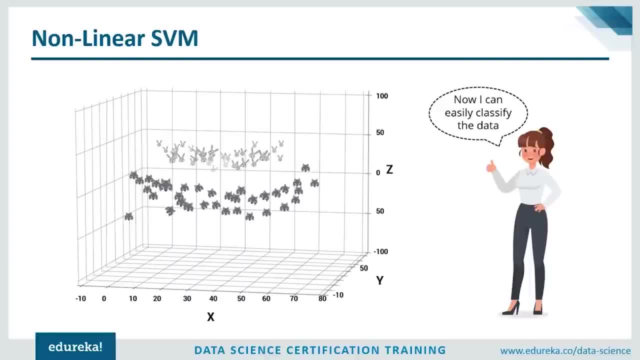 line. All right, in order to deal with such data sets, you're going to transform them into linear Data sets and then use SVM on them. Okay, so a simple trick would be to transform the two variables X and Y into a new feature space involving a new variable called Zed. 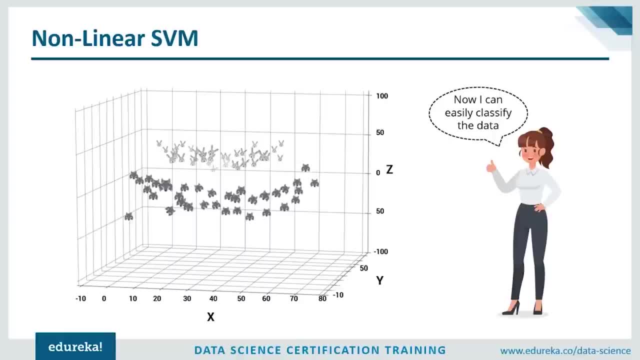 All right. So, guys, so far we were plotting our data on two-dimensional space. Correct, We were only using the X and the y-axis, So we had only those two variables, X and Y. now, in order to deal with this kind of data, a simple trick would be to transform the two variables X and Y. 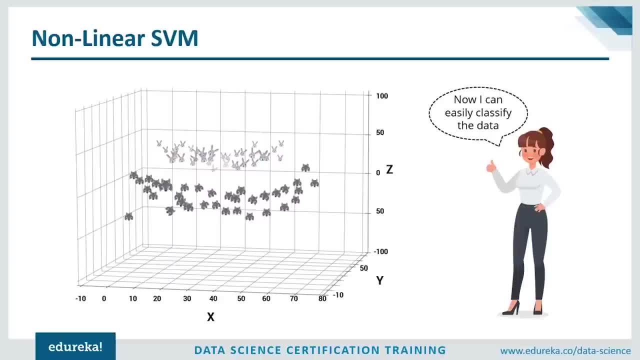 into a new feature Space involving a new variable called Zed. Okay, so we're basically visualizing the data on a three-dimensional space. Now, when you transform the 2D space into a 3D space, you can clearly see a. 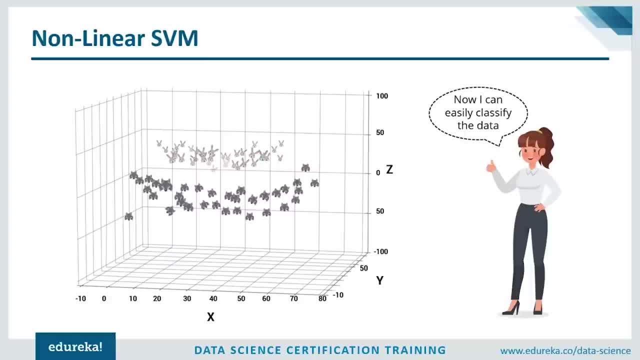 dividing margin between the two classes of data. All right, Now you can go ahead and separate the two classes by drawing the best hyperplane between them. Okay, that's exactly what we discussed in the previous slides. So, guys, why don't you try this yourself? 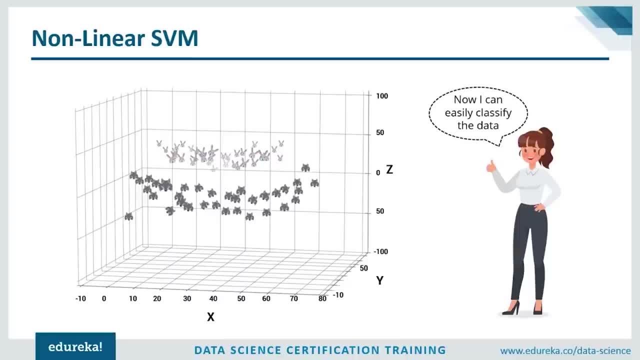 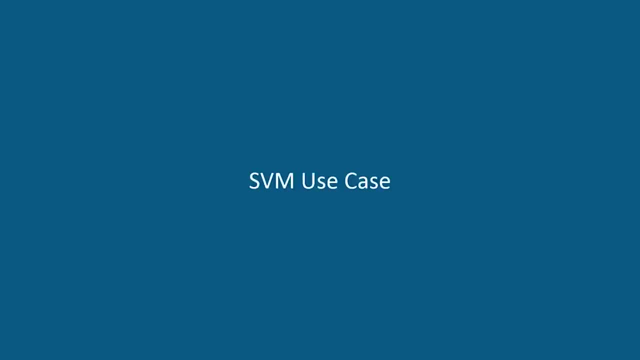 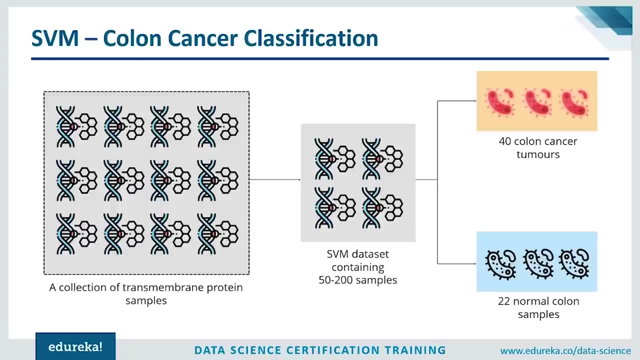 Try drawing a hyperplane which is the most optimum for these two classes. All right, So, guys, I hope you have a good understanding about nonlinear SVMs. Now let's look at a real-world use case of support vector machines. So, guys, SVM as a classifier has been used in cancer classification. 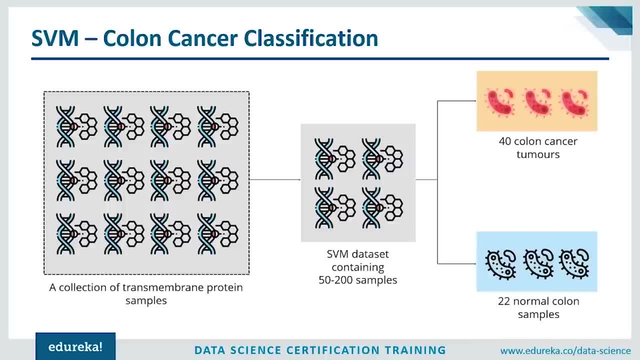 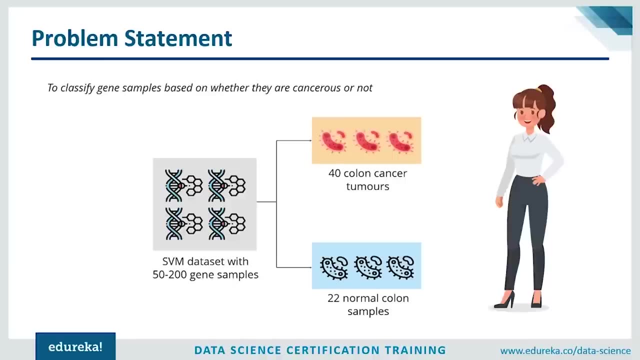 since the early 2000s. So there was an experiment held by a group of professionals who applied SVM in a colon cancer tissue classification. So the data set consisted of about 2,000 transmembrane protein samples and only about 50 to 200 gene samples were input into the SVM classifier. 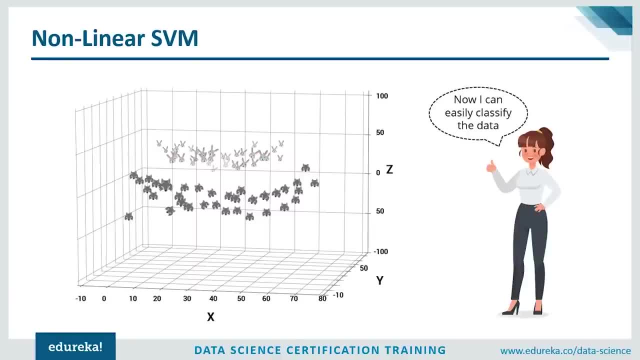 nonlinear spaces into linear ones. Nonlinear data set is the one that you can't separate using a straight line. All right, in order to deal with such data sets, you're going to transform them into linear data sets and then use SVM on them. 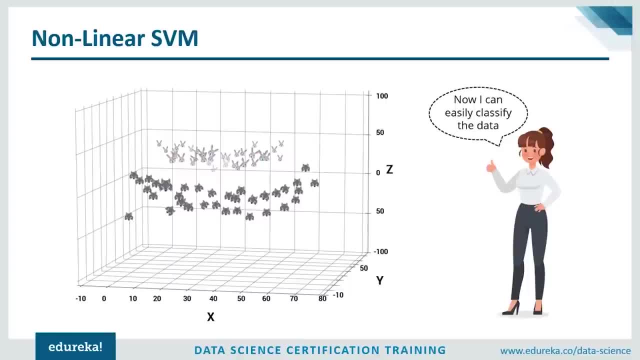 Okay, So a simple trick would be to transform the two variables X and Y Y into a new feature space involving a new variable called Z. All right, so, guys, so far we were plotting our data on two dimensional space, correct. We were only using the X and the y-axis. 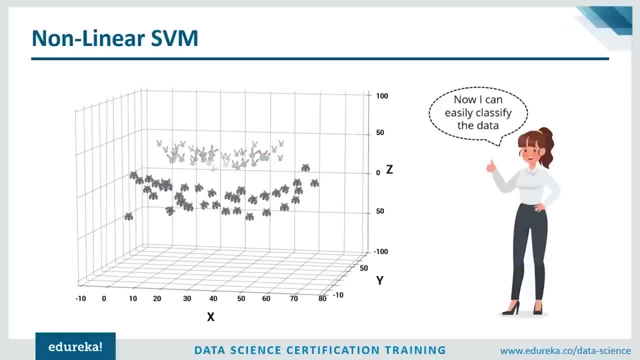 So we had only those two variables, X and Y. Now, in order to deal with this kind of data, a simple trick would be to transform the two variables X and Y into a new feature space involving a new variable called Z. Okay, so we're basically visualizing the data on a three-dimensional. 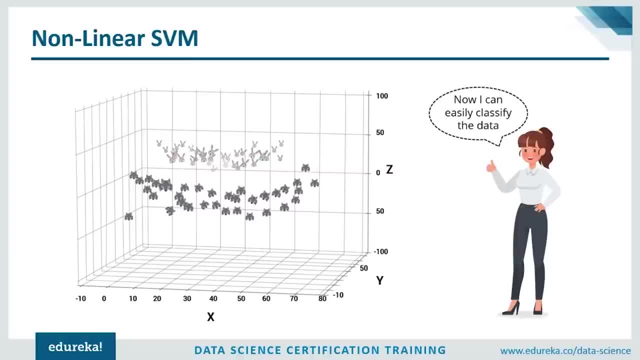 space. Now, when you transform the 2D space into a 3D space, you can clearly see a dividing margin between the two classes of data. All right, Now you can go ahead and separate the two classes by drawing the best hyperplane between them. 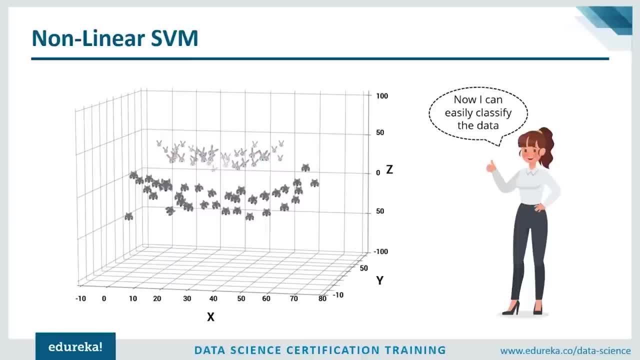 Okay, that's exactly what we discussed in the previous slides. So, guys, why don't you try this yourself? Try drawing a hyperplane which is the most optimum for these two classes. All right, So, guys, I hope you have a good understanding about nonlinear SVMs. 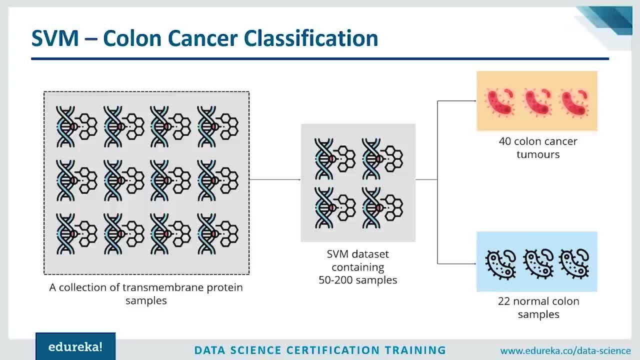 Now let's look at a real-world use case of support vector machines. So, guys, SVM as a classifier has been used in cancer classification since the early 2000s. So there was an experiment held by a group of professionals who applied. 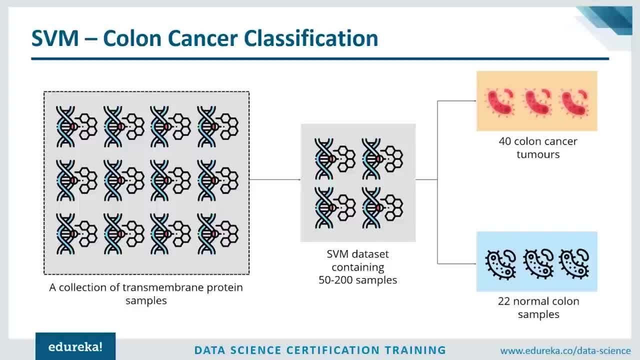 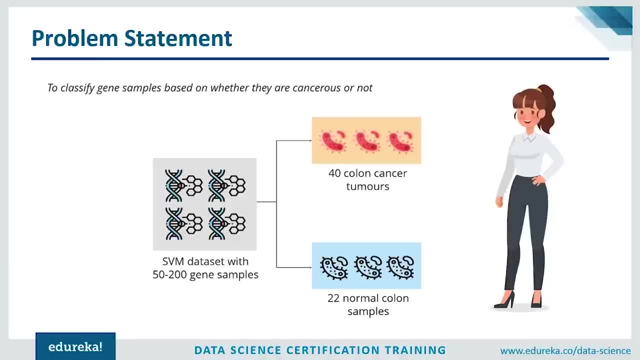 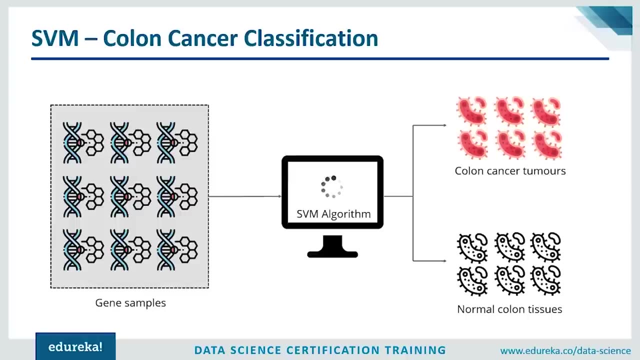 SVM in a colon cancer tissue classification. So the data set consisted of about 2000 transmembrane protein samples and only about 50 to 200 gene samples were input into the SVM classifier. Now this sample which was input into the SVM classifier had both colon cancer tissue samples and normal colon tissue samples. 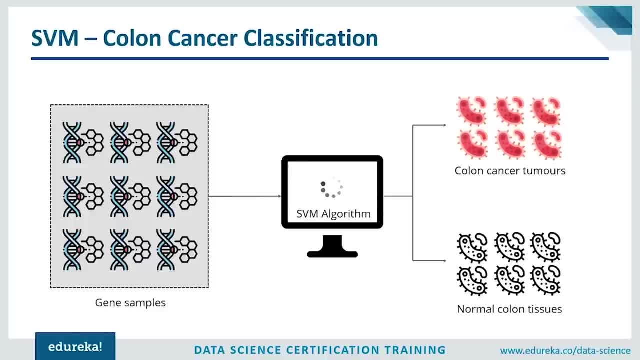 All right Now. the main objective of the study was to classify gene samples based on whether they are cancerous or not. Okay, So SVM was trained using the 50 to 200 samples in order to discriminate between non-tumor from tumor specimens. 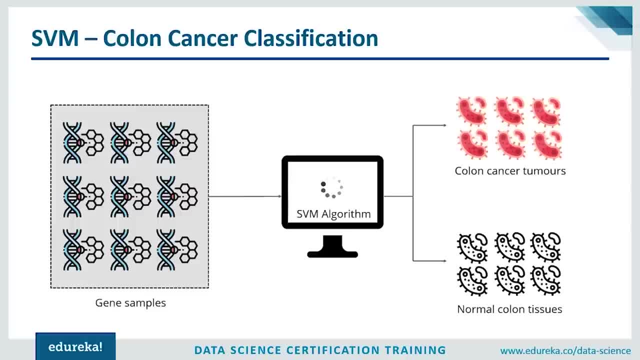 Now, this sample, which was input into the SVM classifier, had both colon cancer tissue samples and normal colon tissue samples. All right Now. the main objective of the study was to classify gene samples based on whether they are cancerous or not. Okay, so SVM was trained using the 50 to 200 samples in order to discriminate. 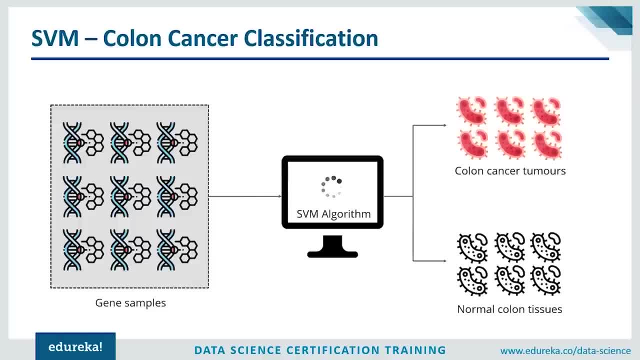 between non-tumor from tumor specimens. So the performance of the SVM classifier was very accurate for even a small data set. All right, We had only 50 to 200 samples and even for the small data set, SVM was pretty accurate with its results. 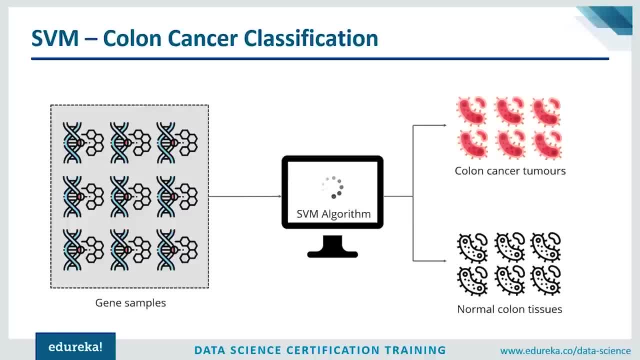 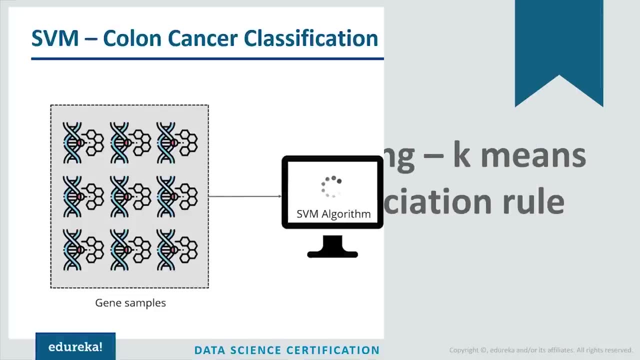 Not only that, its performance was compared to other classification algorithms like naive Bayes, and in each case SVM outperform naive Bayes. So after this experiment, it was clear that SVM classified the data more effectively and it worked exceptionally good with small data sets. 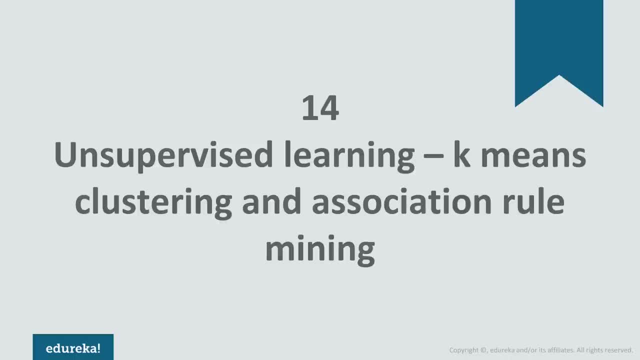 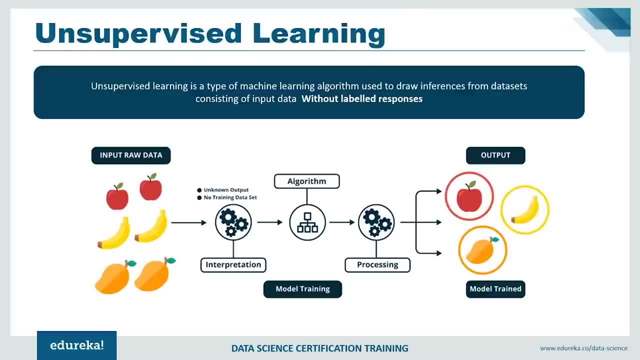 Let's go ahead and understand what exactly is unsupervised learning. So sometimes the given data is unstructured and unlabeled, So it becomes difficult to classify the data into different categories. So unsupervised learning helps to solve this problem. This learning is used to cluster the input data in classes on the basis of: 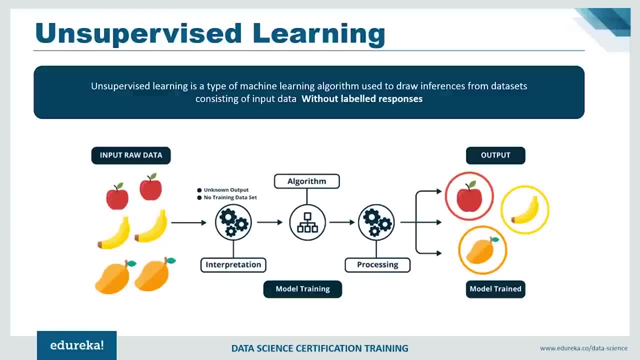 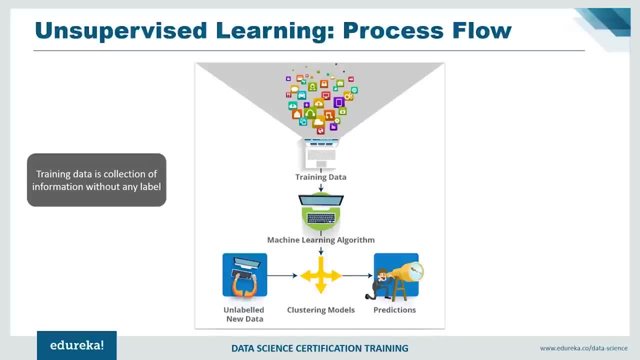 their statistical properties. So, example, we can cluster different bikes based upon the speed limit, their acceleration or the average that they are giving. So unsupervised learning is a type of machine learning algorithm used to draw inferences from data sets consisting of input data without labeled. 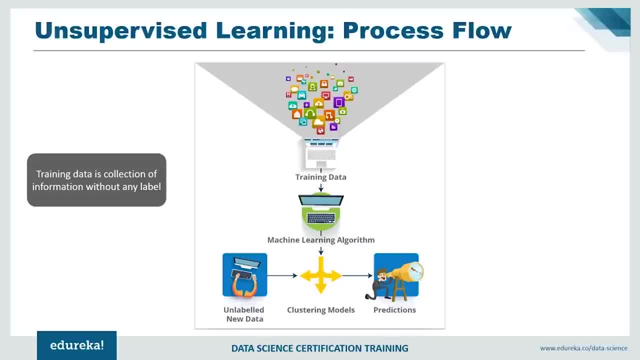 responses. So if you have a look at the workflow or the process flow of unsupervised learning, so the training data is collection of information without any label. We have the machine learning algorithm and then we have the clustering models. So what it does is that distributes the data into different clusters. 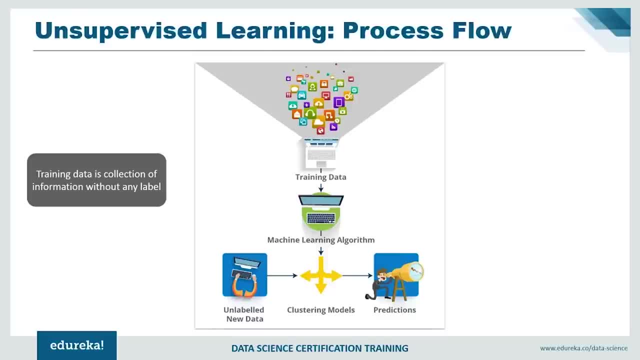 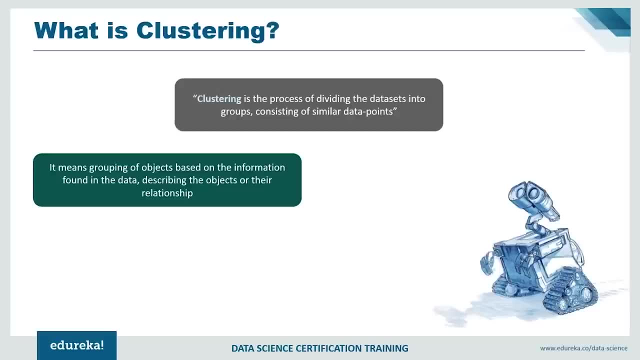 And again, if you provide any unlabeled new data, it will be able to make a prediction and find out to which cluster that particular data or the data set belongs to or the particular data point belongs to. So one of the most important algorithms in unsupervised learning is clustering. 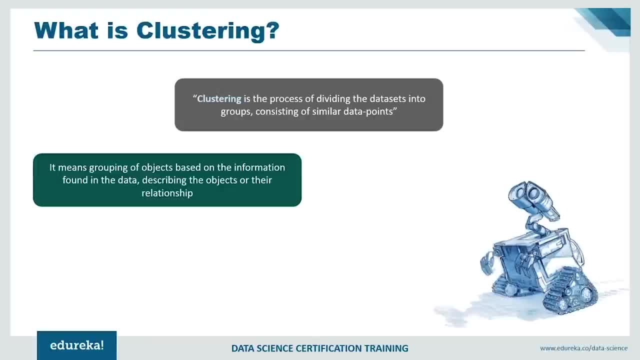 So let's understand exactly what is clustering. So clustering, basically, is the process of dividing the data sets into groups consisting of similar data points. It means grouping of objects based on the information found in the data describing the objects or their relationships. So clustering models. 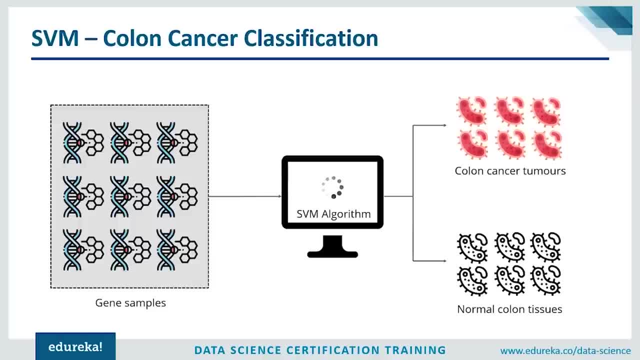 So the performance of the SVM classifier was very accurate for even a small data set. All right, we had only 50 to 200 samples and even for the small data set, SVM was pretty accurate with its results. Not only that, its performance was compared to other classification. 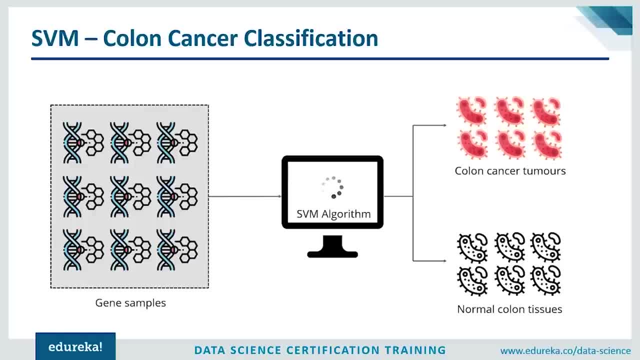 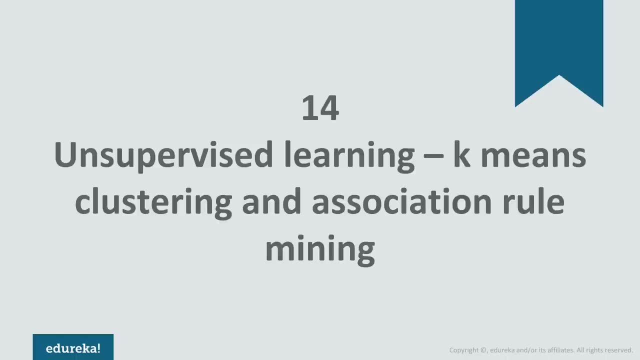 algorithms like naive Bayes and in each case, SVM outperform naive Bayes. So after this experiment, it was clear that SVM classified the data more effectively and it worked exceptionally good with small data sets. Let's go ahead and understand what exactly is unsupervised learning. 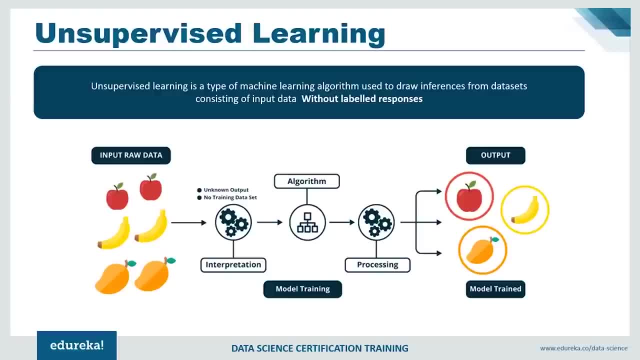 So sometimes Given data is unstructured and unlabeled, So it becomes difficult to classify the data into different categories. So unsupervised learning helps to solve this problem. This learning is used to cluster the input data in classes on the basis of their statistical properties. 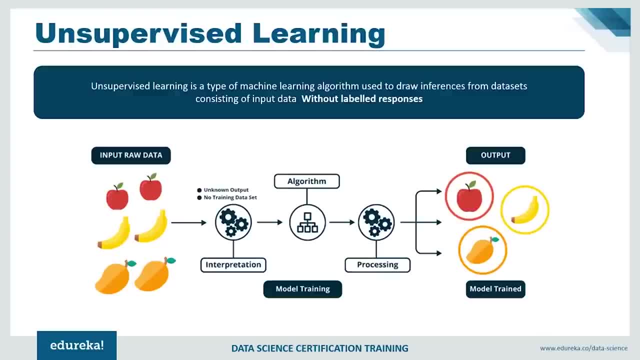 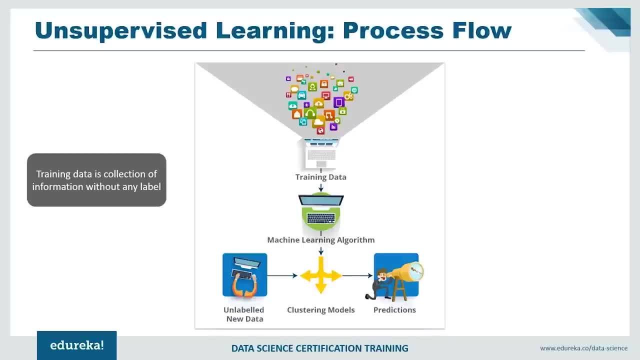 So, example, we can cluster different bikes based upon the speed limit, their acceleration or the average that they are giving. So unsupervised learning is a type of machine learning algorithm used to draw inferences from data sets consistent Of input data without labeled responses. 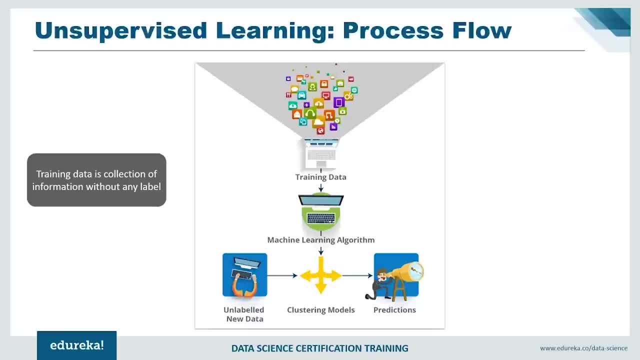 So if you have a look at the workflow or the process flow of unsupervised learning, so the training data is collection of information without any label. We have the machine learning algorithm and then we have the clustering models. So what it does is that distributes the data into different clusters. 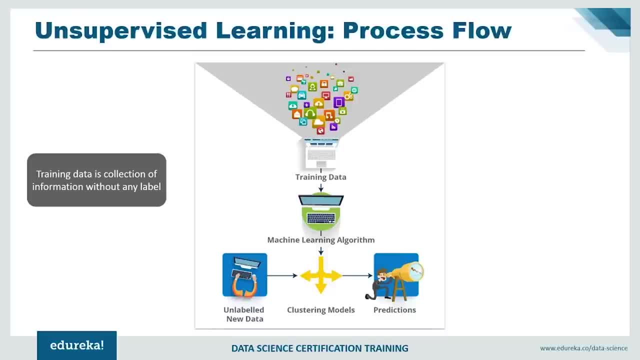 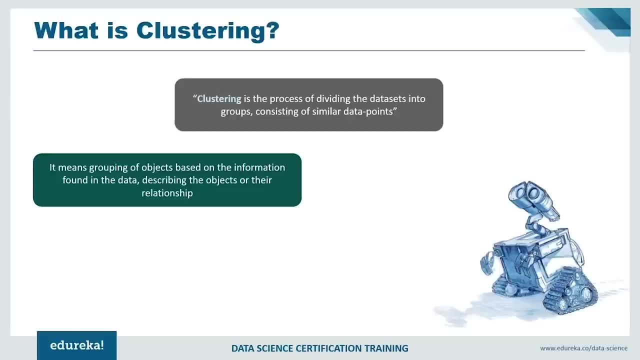 And again, if you provide any unlabeled new data, it will make a prediction and find out to which cluster that particular data or the data set belongs to or the particular data point belongs to. so One of the most important algorithms in unsupervised learning is clustering. 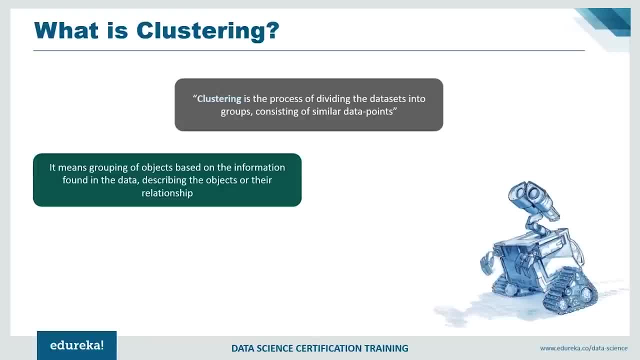 So let's understand exactly what is clustering. So clustering, basically, is the process of dividing the data sets into groups consisting of similar data points. It means grouping of objects based on the information found in the data describing the objects or their relationships. So clustering models focus on identifying groups of similar records and 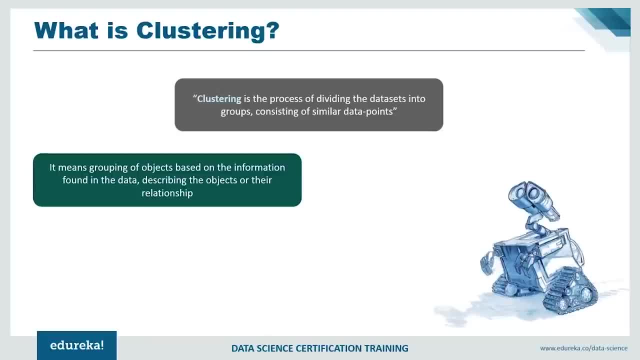 Focus on identifying groups of similar records and labeling records according to the group to which they belong. Now, this is done without the benefit of prior knowledge about the groups and their characteristics. So, and in fact we may not even know exactly how many groups are there to. 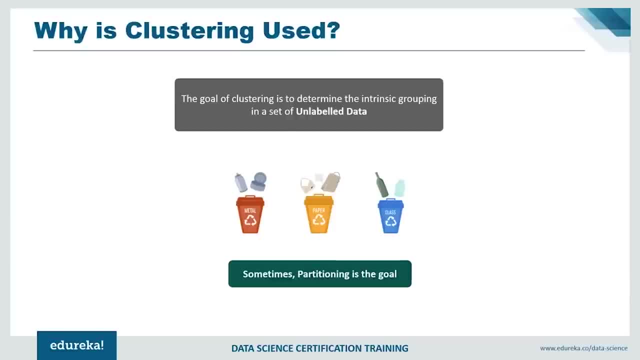 look for. Now. these models are often referred to as unsupervised learning models. since there is no external standard by which to judge the models classification performance, There are no right or wrong answers to these models, And if we talk about why clustering is used, so the goal of clustering is 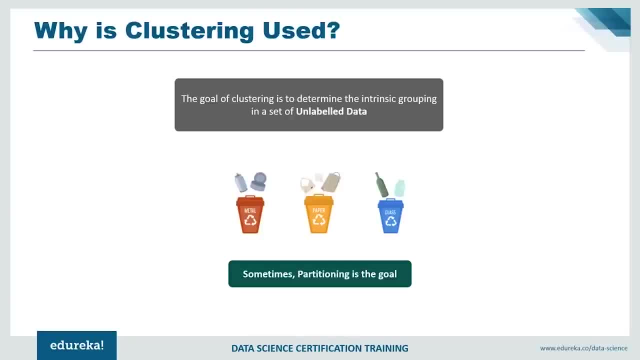 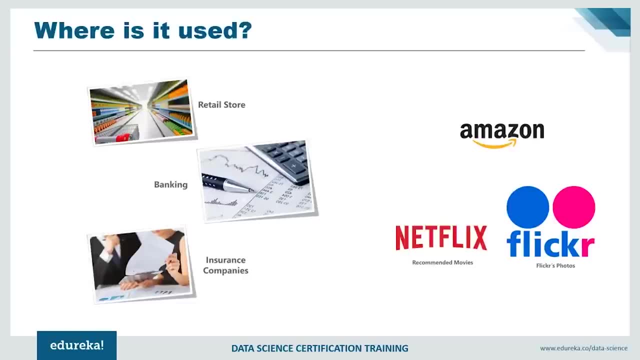 to determine the intrinsic group in a set of unlabeled data. Sometimes the partitioning is the goal or the purpose of clustering algorithm is to make sense of and exact value from the last set of structured and unstructured data. So that is why clustering is used in the industry. 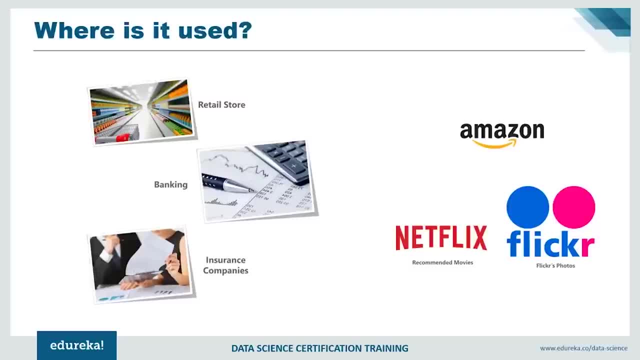 And if you have a look at the various use cases of clustering in the industry, so first of all, it's being used in marketing. So discovering distinct groups in customer databases, such as customers who make a lot of long-distance calls, customers who use internet more than. 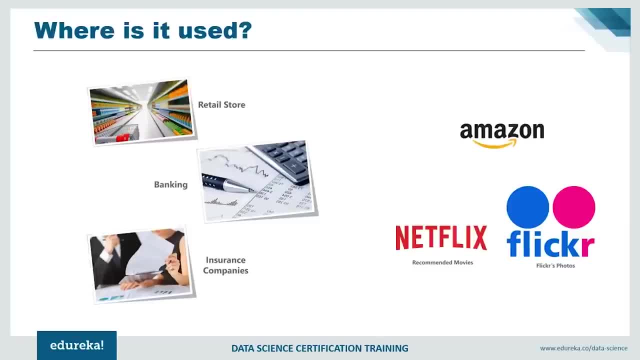 cause. they also use an insurance companies for, like identifying groups of corporation insurance policy holders with high average claim rate. farmers crash cops, which is profitable. They are using seismic studies and define probable areas of oil or gas exploration based on seismic data, And they're also used in the recommendation of movies. 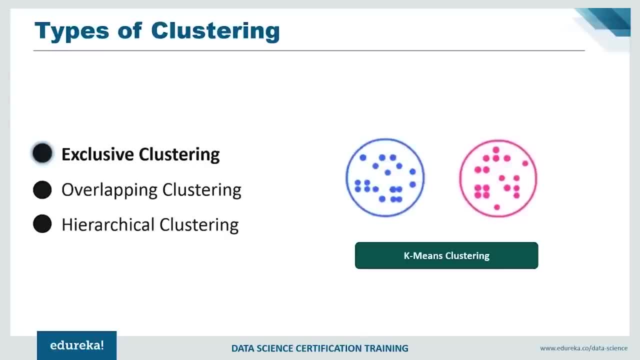 If you would say, they are also used in Flickr photos. They also use by Amazon for recommending the product which category it lies in. So basically, if we talk about clustering, there are three types of clustering. So first of all we have the exclusive clustering, which is the hard clustering. 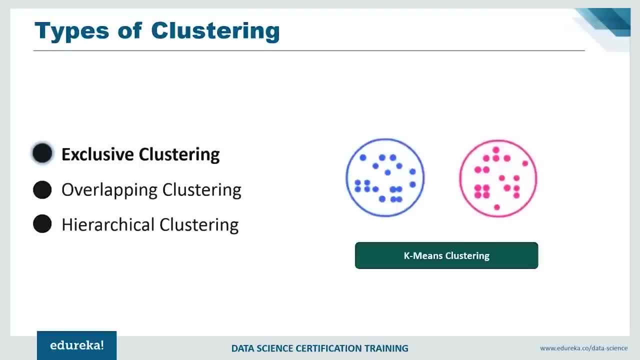 So here an item belongs exclusively to one cluster, not several clusters, and the data point belong exclusively to one cluster. So an example Of this is the came in clustering, So came in clustering. does this exclusive kind of clustering? So secondly, we have overlapping clustering. 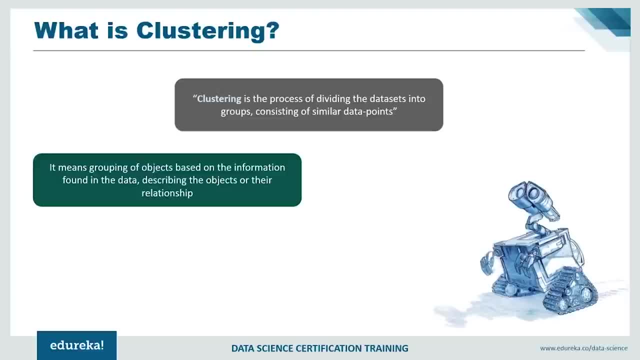 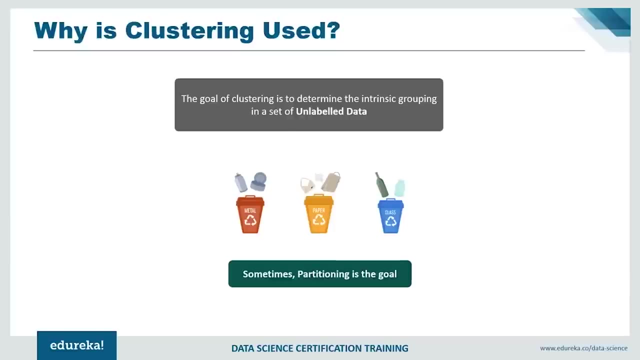 labeling records according to the group to which they belong. Now, this is done without the benefit of prior knowledge about the groups and their characteristics. So, and in fact, we may not even know exactly how many groups are there to look for. Now, these models are often referred to as unsupervised learning models. 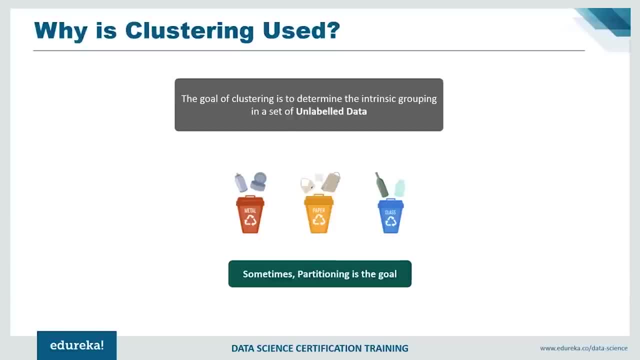 since there is no external standard by which to judge the models classification performance, There are no right or wrong answers to these model. And if we talk about why clustering is used. so the goal of clustering is to determine the intrinsic group in a set of unlabeled data. 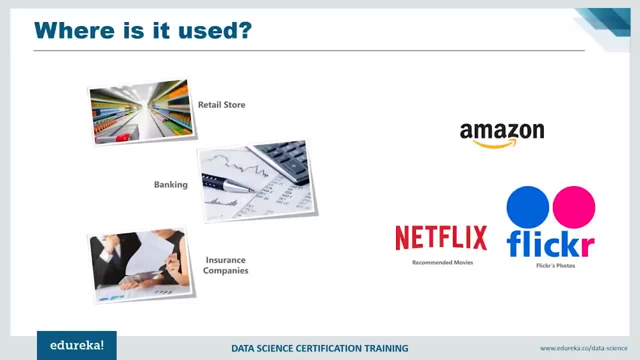 Sometimes the partitioning is the goal or the purpose of clustering algorithm is to make sense of and exact value from the last set of structured and unstructured data. So that is why clustering is used in the industry, And if you have a look at the various use cases of clustering in the 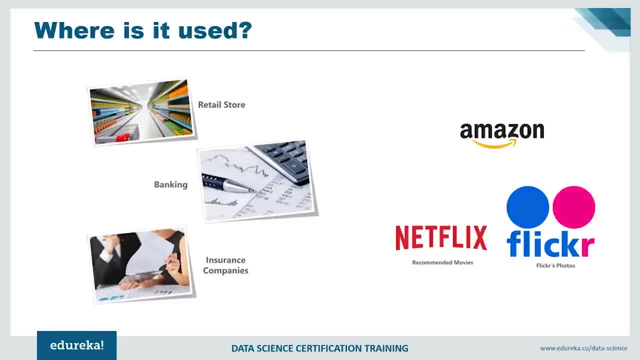 industry. so, first of all, it's being used in marketing. So discovering distinct groups in customer databases, such as customers who make a lot of long-distance calls, customers who use internet more than calls. They're also using insurance companies like identifying groups of. 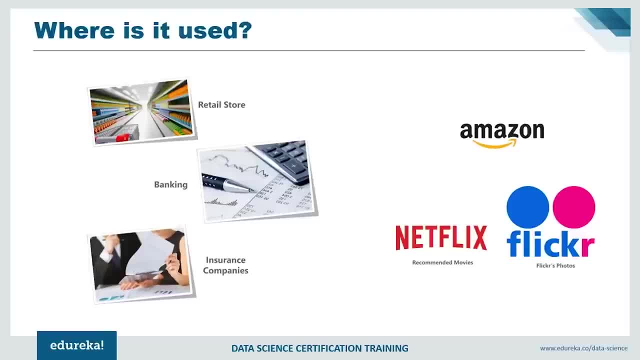 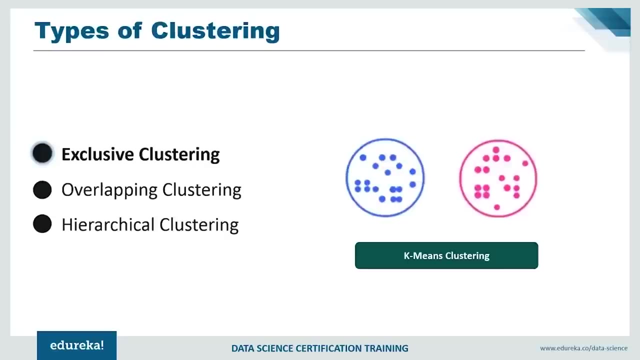 corporation insurance policy holders with high average claim rate. farmers crash cops, which is profitable. They are using seismic studies and define probable areas of oil or gas exploration based on seismic data, And they're also used in the recommendation of movies, if you'd say. 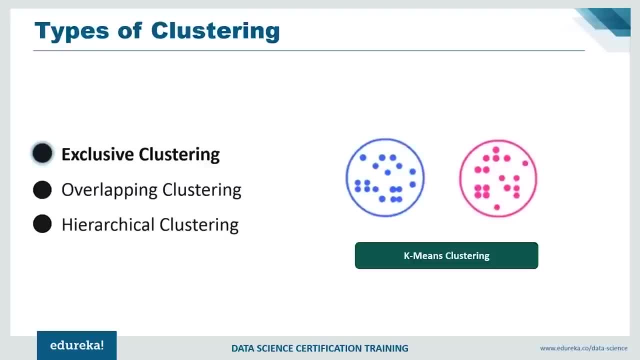 they are also used in Flickr photos. they also used by Amazon for recommending the product, which category it lies in. So basically, if we talk about clustering, there are three types of clustering. So first of all, we have the exclusive clustering, which is the hard. 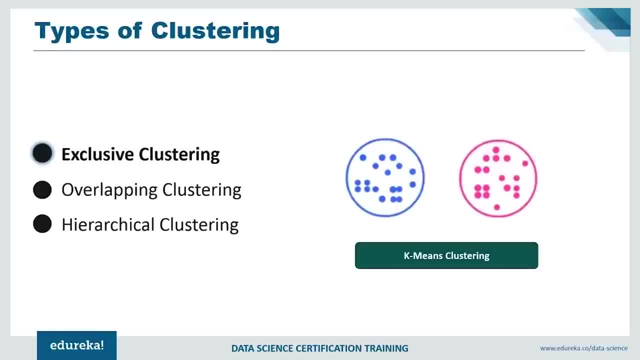 clustering. So here an item belongs exclusively to one cluster, not several clusters, and the data point belong exclusively to one cluster. So an example of this is the K-Mean clustering. So K-Mean clustering does this exclusive kind of clustering. So secondly, we have overlapping clustering. 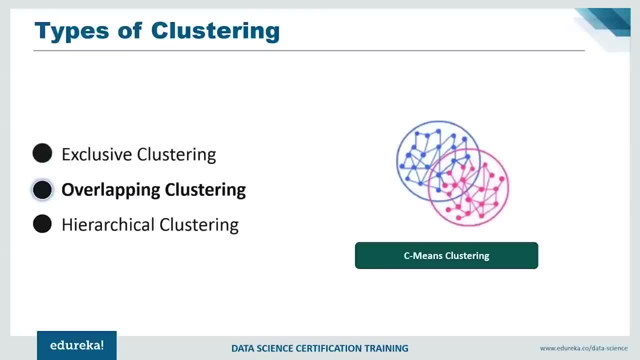 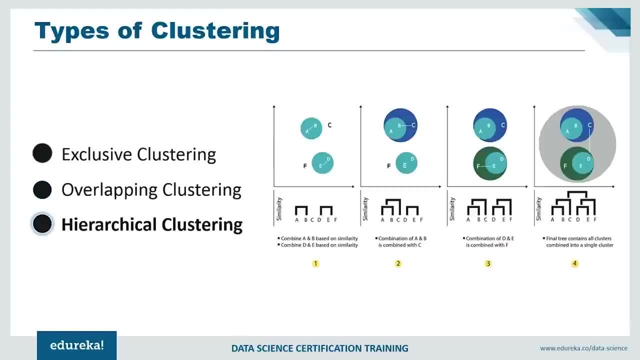 So it is also known as soft clusters. In this, an item can belong to multiple clusters as its degree of association with each cluster is shown, And for example, we have fuzzy or the C-Means clustering, which is being used for overlapping clustering. 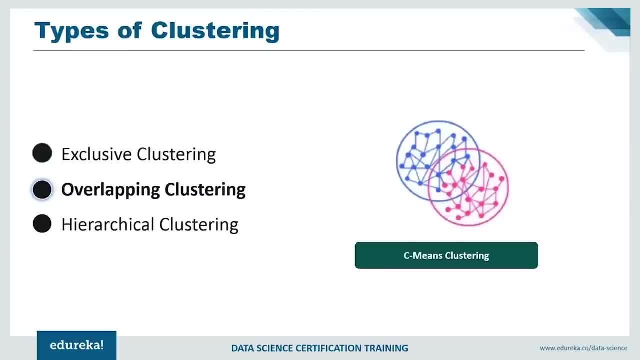 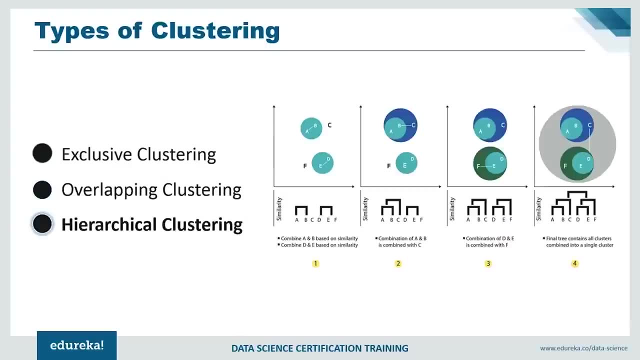 So it is also known as soft clusters. in this an item can belong to multiple clusters as its degree of association with each cluster is shown. And for example, we have fuzzy or the C means clustering which is being used for overlapping clustering, And finally we have the hierarchical clustering. 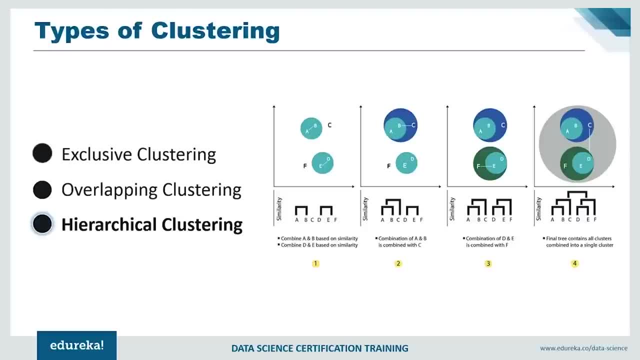 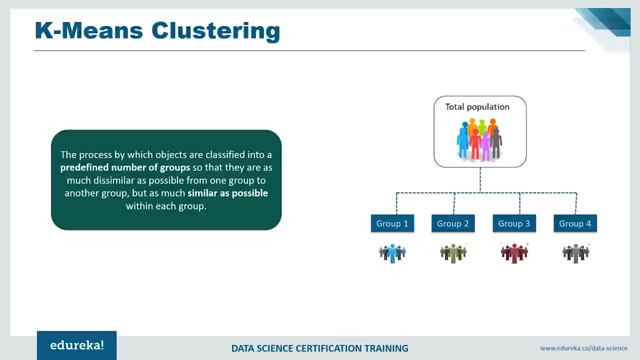 So when two clusters Have a parent-child relationship or a tree-like structure, then it is known as hierarchical cluster. So as you can see here from the example, we have a parent-child kind of relationship in the cluster given here. So let's understand what exactly is K means clustering? 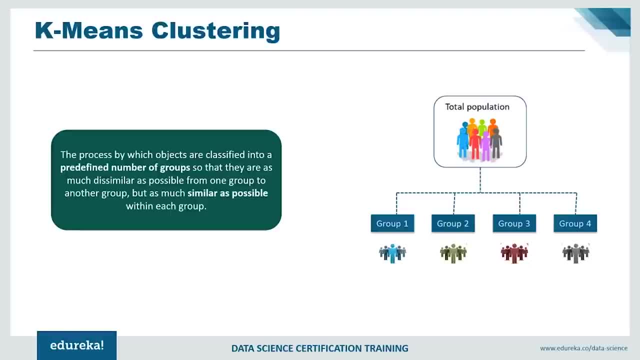 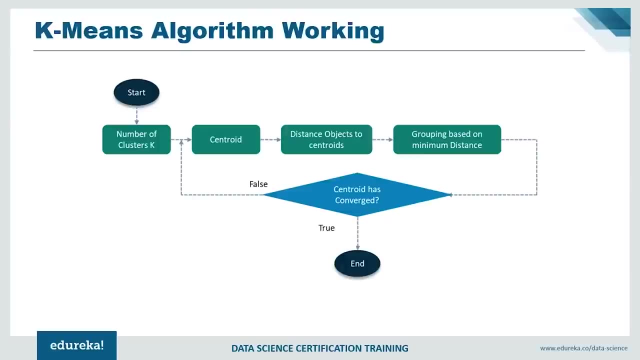 So K means clustering- is an algorithm whose main goal is to group similar elements of data points into a cluster, and it is the process by which objects are classified into a predefined number of groups so that they are as much Just, similar as possible from one group to another group, but as much as similar or possible. 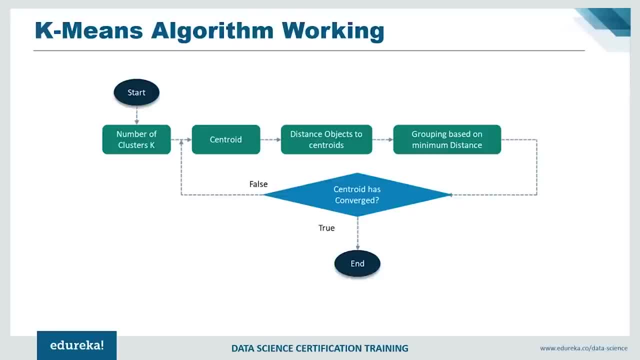 within each group. Now, if you have a look at the algorithm working here, you're right. So first of all, it starts with identifying the number of clusters, which is key. Then again we find the centroid. We find the distance objects to the distance object to the centroid. distance of objects to the 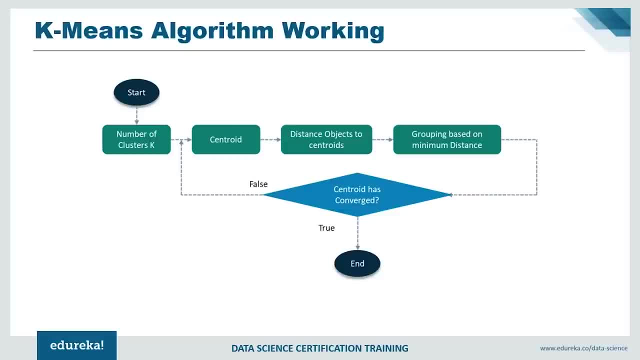 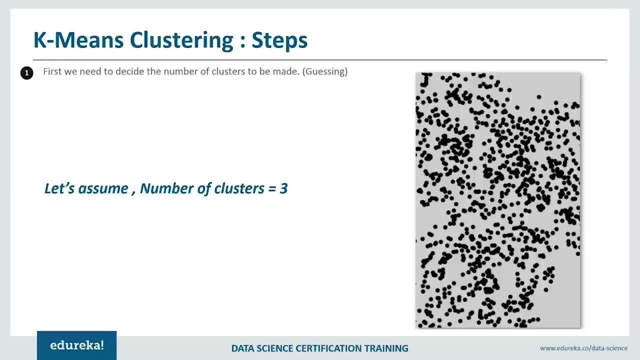 centroid. Then we find the grouping based on the minimum distance. has the centroid? Centroid converts? If true, then we make a cluster. If false, we then again find the centroid. repeat all of the steps again and again. So let me show you how exactly clustering was with an example here. 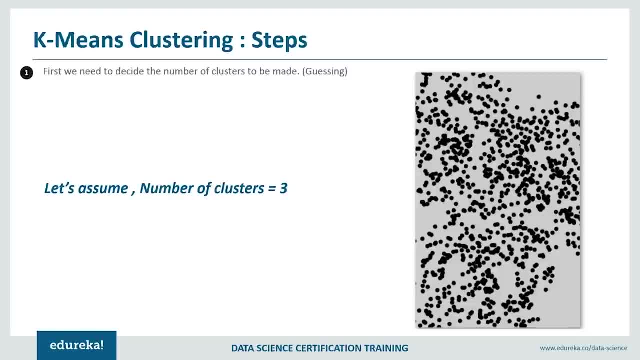 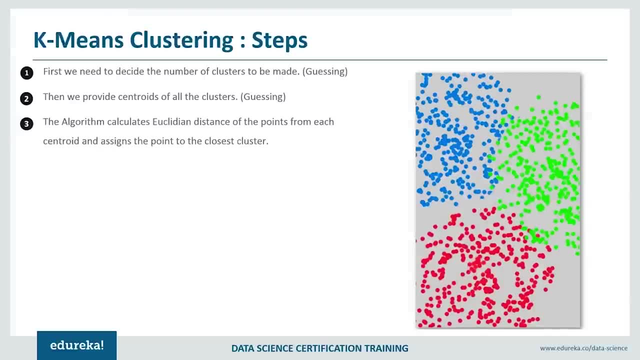 So first we need to decide the number of clusters to be made Now. another important task here is how to decide the number of clusters, or how to decide the number of clusters. We'll get into that later. So first let's assume that the number of clusters we have decided is three. 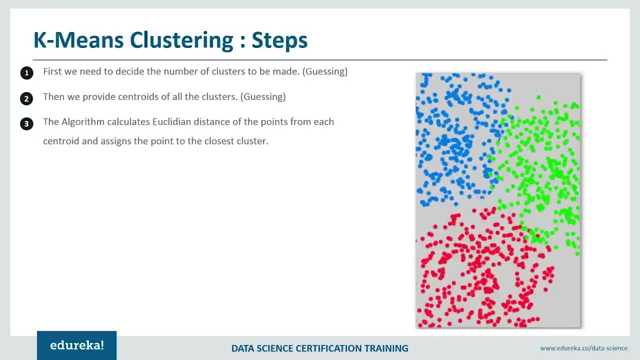 So after that, then, we provide the centroid for all the clusters. which is guessing? the algorithm calculates the Euclidean distance of the point from each centroid and assigns the data point to the closest cluster. Now, Euclidean distance, all of you know, is the square root of the distance, the square root of. 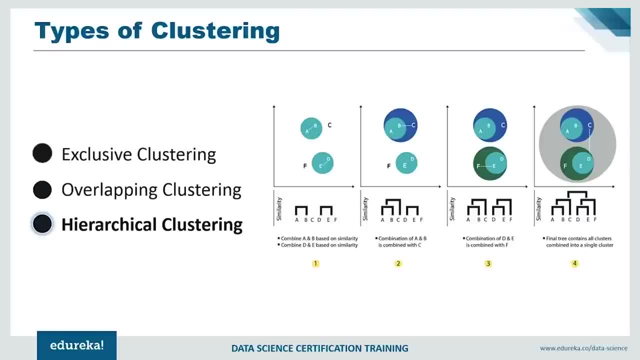 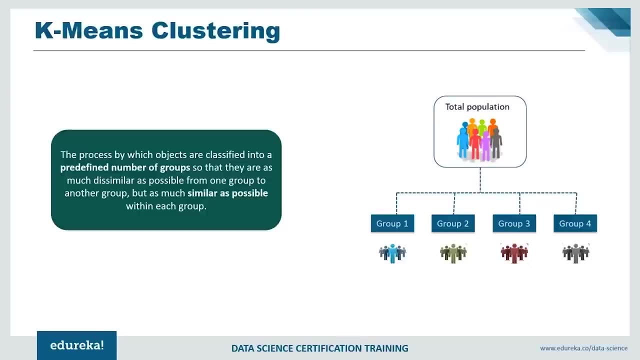 And finally we have the hierarchical clustering. So when two clusters have a parent-child relationship or a tree-like structure, then it is known as hierarchical clustering. So as you can see here from the example, we have a parent-child kind of relationship in the cluster given here. 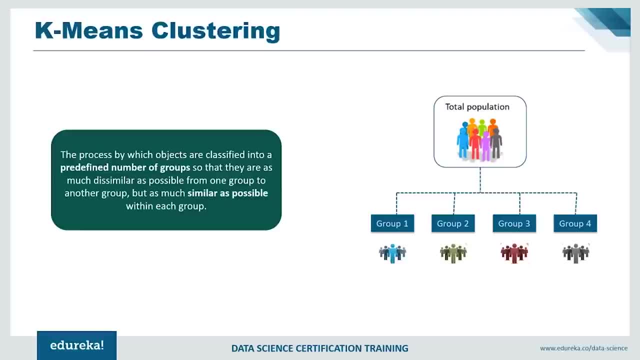 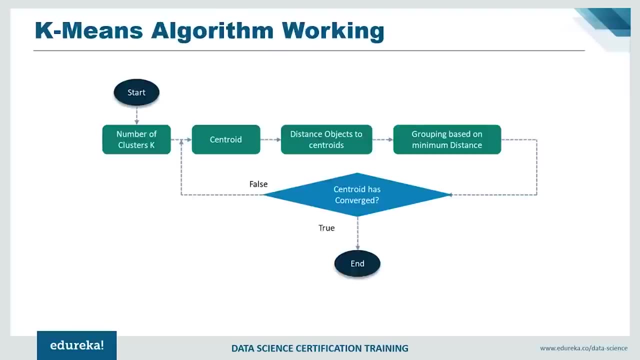 So let's understand what exactly is K-Means clustering. So K-Means clustering is an algorithm whose main goal is to group similar elements of data points into a cluster, And it is the process by which objects are classified into a predefined number of groups so that they are as much dissimilar as possible from. 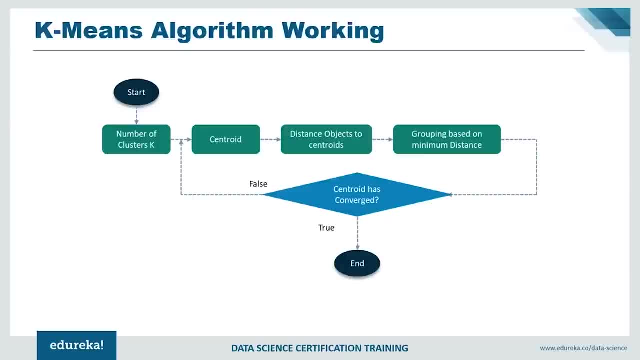 one group to another group, but as much as similar Or possible within each group. Now, if you have a look at the algorithm working here, you're right. So first of all, it starts with identifying the number of clusters, which is K. Then again we find the centroid. 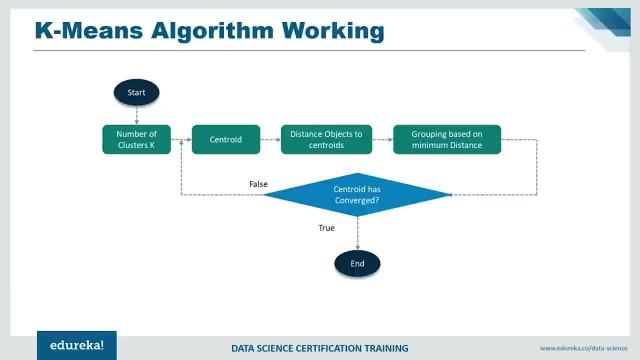 We find the distance. objects to the distance, object to the centroid, distance of objects to the centroid. Then we find the grouping based on the minimum distance. Has the centroid converged? If true, then we make a cluster. If false, we then again find the centroid. 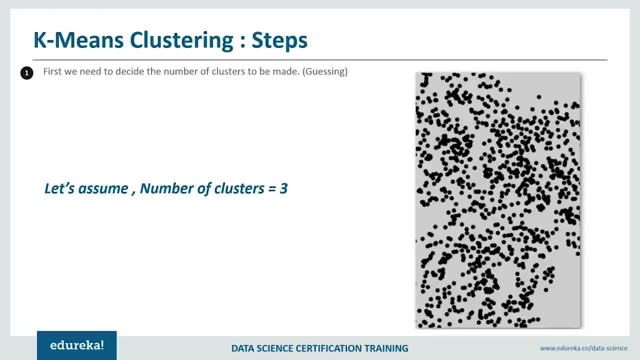 Repeat all of the steps again and again. So let me show you how exactly clustering was with an example here. So first we need to decide the number of clusters to be made. Now. another important task here is how to decide the number of clusters, or how to decide the number of clusters. 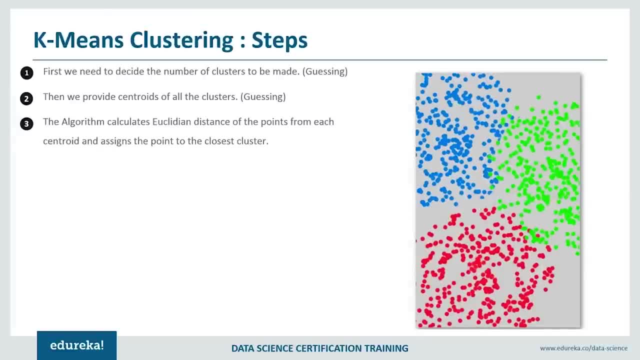 We'll get into that later. So first let's assume that the number of clusters we have decided is three. So after that, then, we provide the centroid for all the clusters, which is guessing, And the algorithm calculates the Euclidean distance of the point from each. 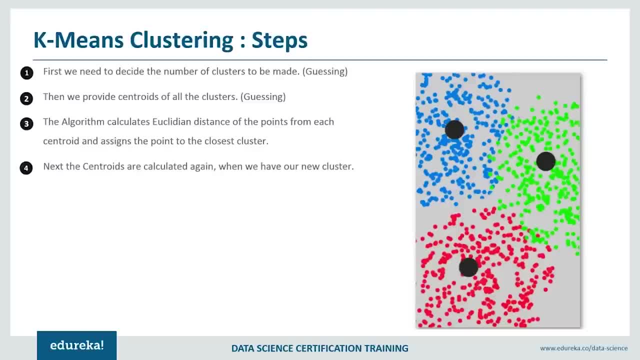 centroid and assigns the data point to the closest cluster. Now, Euclidean distance, all of you know, is the square root of the distance, the square root of the square of the distance. So next, when the centroids are calculated again, we have our new. 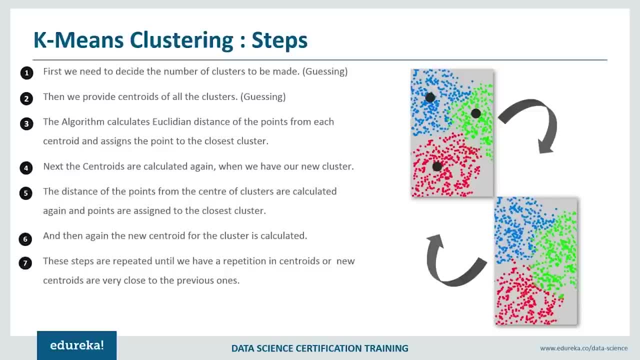 clusters for each data point. Then again the distance from the points to the new clusters are calculated, And then again the points that are assigned to the closest cluster, And then again we have the new centroid is calculated. Now these steps are repeated until we have a repetition in the centroids. 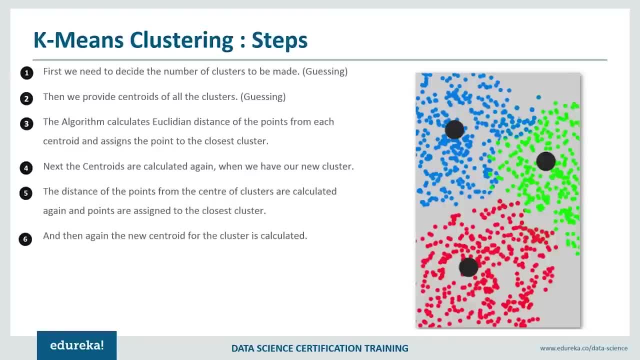 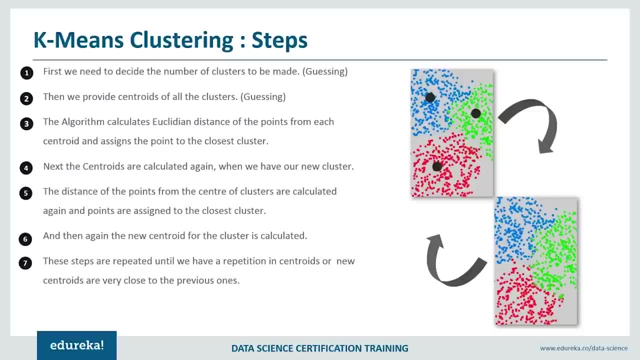 the square of the distance. So next, when the centroids are calculated again, we have our new clusters for each data point, Then again the distance from the points to The new clusters are calculated, And then again the points that are assigned to the closest cluster. 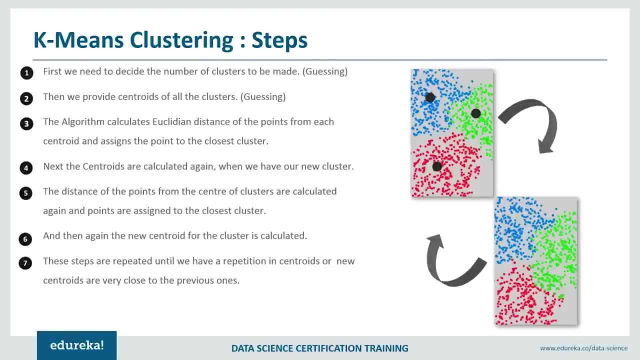 And then again we have: the new centroid is calculated. Now these steps are repeated until we have a repetition in the centroids or the new centroid are very close to the very previous ones. So until and unless our output gets repeated or the outputs are very, very close enough, 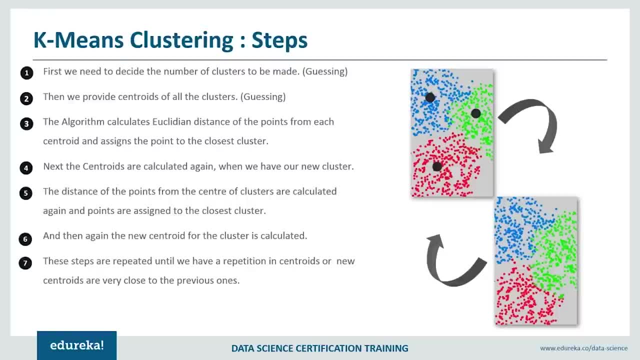 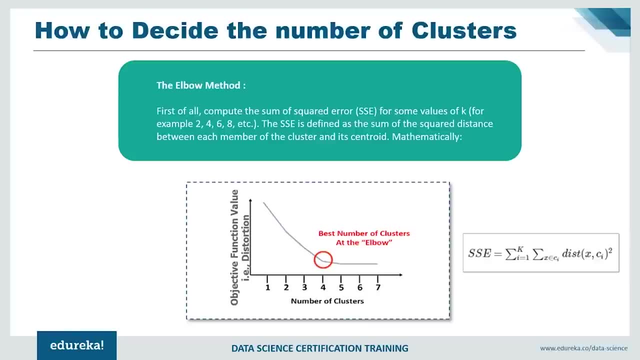 we do not stop this process. We keep on calculating the Euclidean distance of all the points to the centroids, then we calculate, calculate the new centroids, and that is how claim means clustering works basically. so an important part here is to understand how to decide the value of k or the number of clusters, because 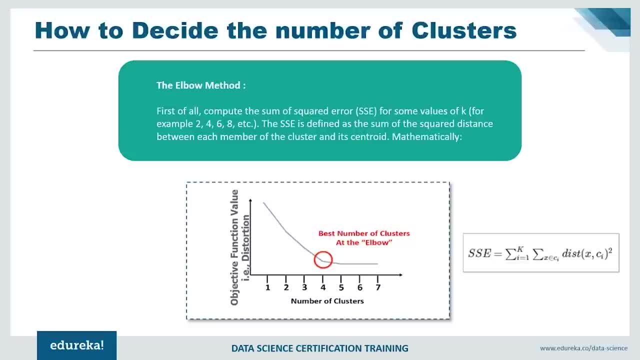 it does not make any sense if you do not know how many clusters you're going to make. so to decide the number of clusters we have the elbow method. so let's assume first of all compute the sum squared error, which is the sse for sum value of a. for example, let's take 2, 4, 5 and 8. now the sse. 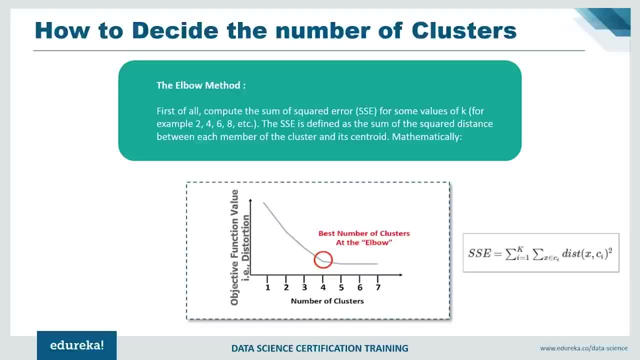 which is the sum squared error, is defined as a sum of the squared distance between each number member of the cluster and its centroid. mathematically, and if you, mathematically it is given by the equation which is provided here, and if you brought the k against the sse, you will. 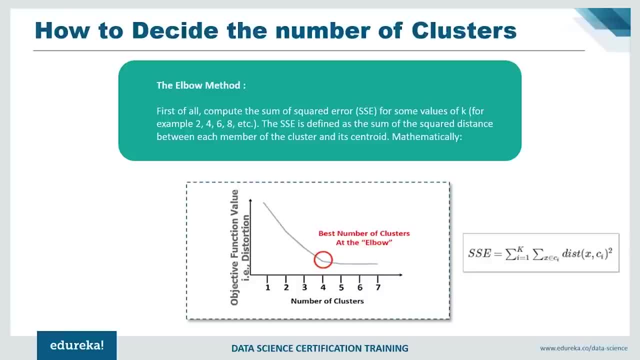 see that the error decreases as k gets large. now this is because of the mドl and theه. the number of cluster increases. they should be smaller, so the distortion is also smaller now. the idea of the elbow method is to choose the key at which the 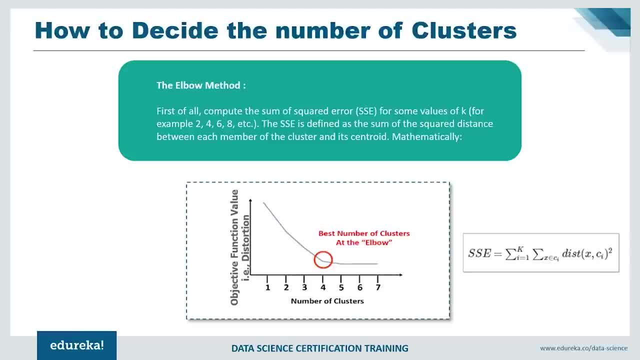 SSE decreases abruptly. so for example here, if we have a look at the figure given here, we see that the best number of cluster is at the elbow. so as you can see here, the graph here changes abruptly after the number four. so for this particular example we're going to use four as a number of cluster. so first of 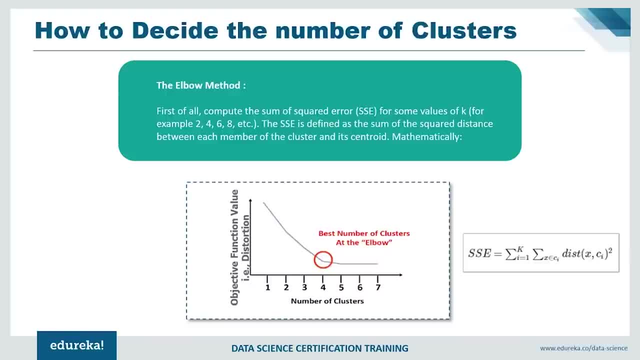 all while working with k-means clustering, there are two key points to know. first of all, be careful about where you start. so choosing the first center at random, choosing the second center that is far away from the first center. similarly, choosing the nth center as far away possible from the closest of the 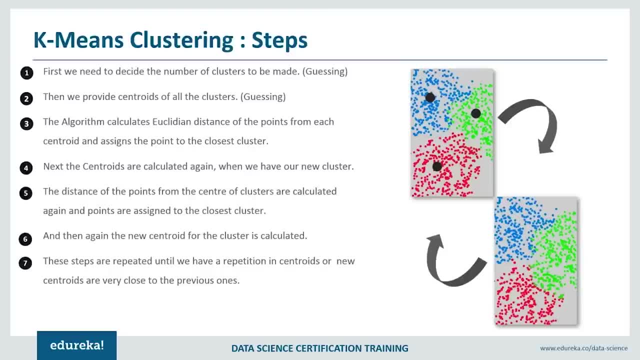 or the new centroids are very close to the very previous ones. So, until and unless our output gets repeated or the outputs are very, very close enough, we do not stop this process. We keep on calculating the Euclidean distance of all the points to the 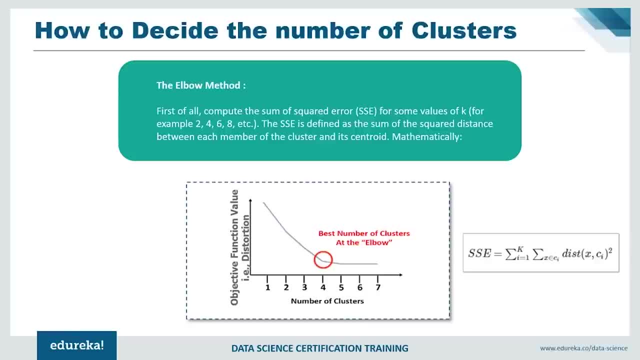 centroids, Then we calculate the new centroids and that is how K-means clustering works basically. So an important part here is to understand how to decide the value of K or the number of clusters, because it does not make any sense if you do not know how many clusters you're going to make. 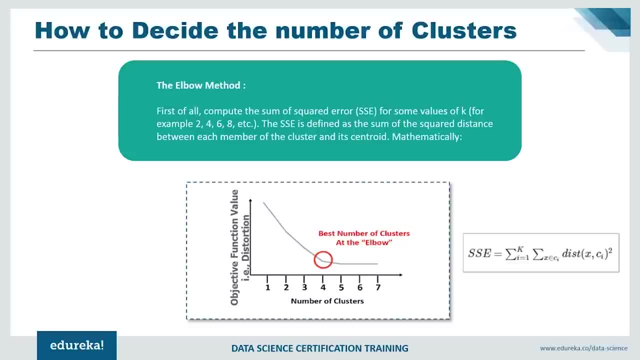 So to decide the number of clusters we have the Elbow method. So let's assume, first of all compute the sum squared error, which is the SSE, for some value of K. For example, let's take 2,, 4,, 6 and 8.. 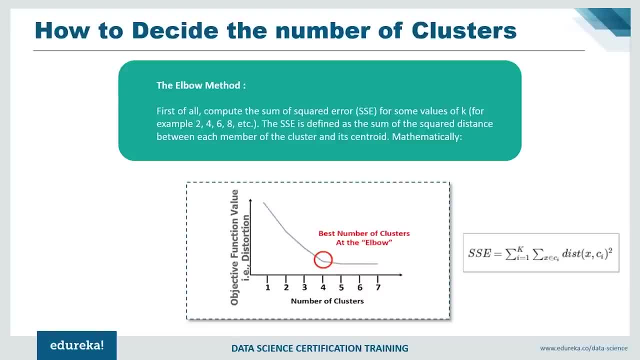 Now the SSE, which is the sum squared error, is defined As a sum of the squared distance between each number member of the cluster and its centroid mathematically. and if you, mathematically it is given by the equation which is provided here, And if you plot the K against the SSE, you will see that the error 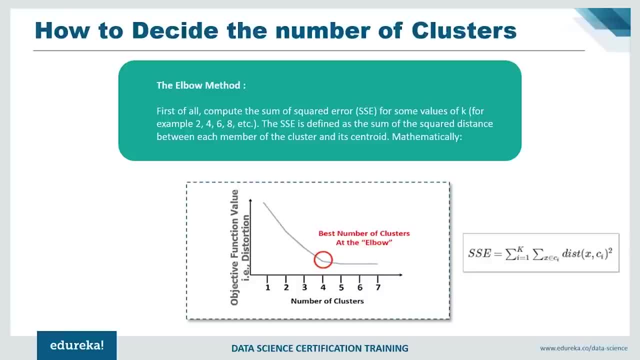 decreases as K gets large. Now this is because the number of cluster increases. they should be smaller, So the distortion is also smaller. Now the idea of the Elbow method is to choose the K at which the SSE increases abruptly. So for example here: if we have a look at the figure given here, we see 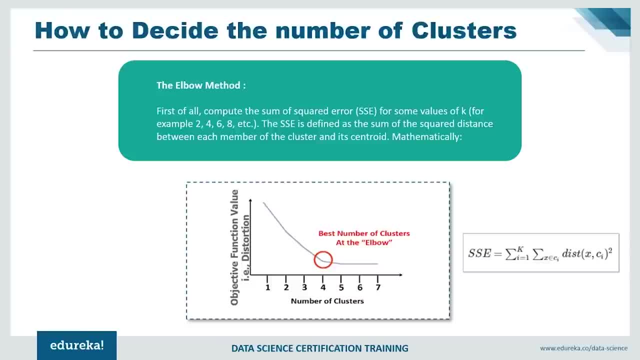 that the best number of cluster is at the Elbow. So, as you can see here, the graph here changes abruptly after the number 4.. So for this particular example, we're going to use 4 as the number of cluster. So first of all, while working with K-Means clustering, there are two key. 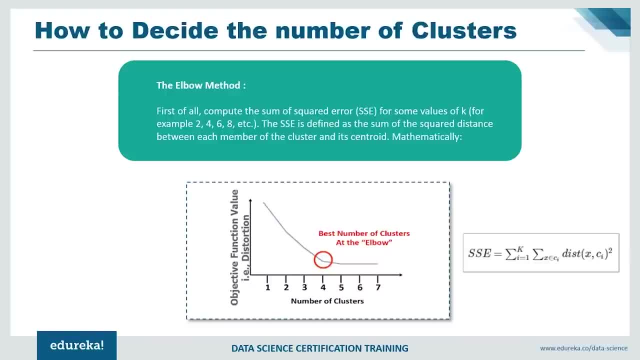 points to know. First of all, be careful about where you start. So choosing the first center at random, Choosing the second center that is far away from the first center. Similarly, choosing the nth center as far away possible from the closest of all the other centers. 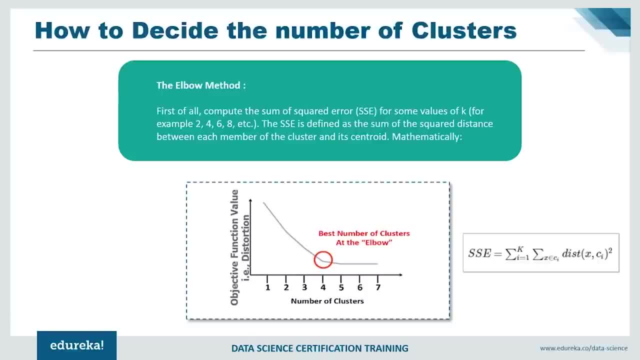 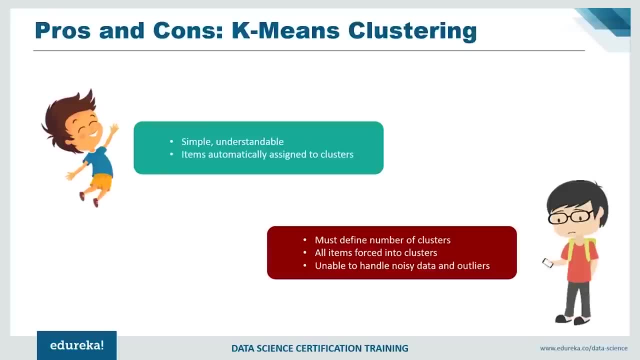 And the second idea is to do as many runs of K-Means, each with different random starting points, so that you get an idea of where exactly and how many clusters you need to make and where exactly the centroid lies and how the data is getting converged. 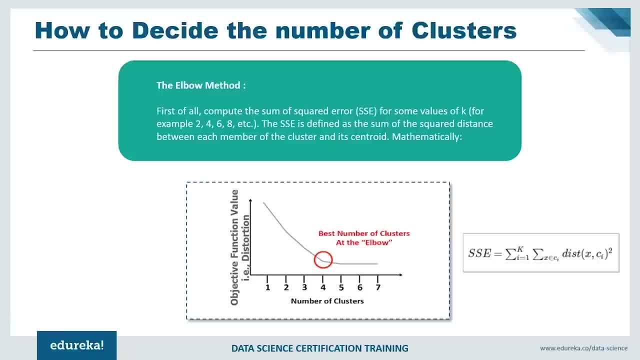 all the other centers. and the second idea is to do as many runs of k-means, each with different random numbers starting points, so that you get an idea of where exactly and how many clusters you need to make and where exactly the centroid lies and how the data is. 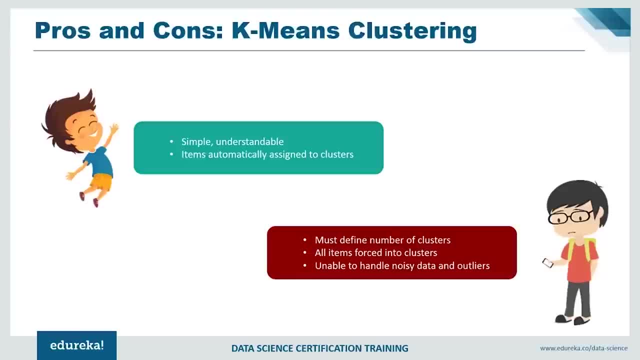 getting converged now k-means is not exactly a very good method. so let's understand the pros and cons of k-means clustering. we know that k-means is simple and understandable. everyone learns it at the first go. the items automatically assigned to the clusters. now, if we have a look at the cons, so 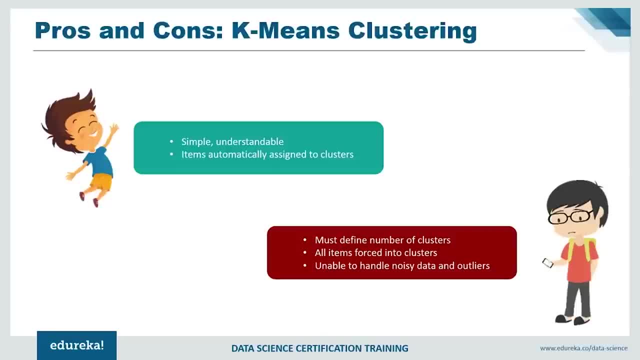 first of all, one needs to define the number of clusters. this is a very heavy task, as us, if we have three, four, or if we have ten categories, and if we do not know what the number of clusters are going to be, it's very difficult for anyone to, you know, to guess the number of clusters now. 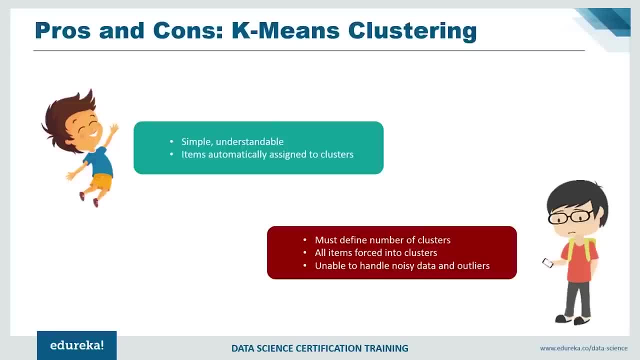 all the items are forced into the clusters, whether they are actually belong to any other cluster or any other category. they are forced to to lie in that other category in which they are closest to now. this again happens because of the number of clusters, with not defining the correct number of. 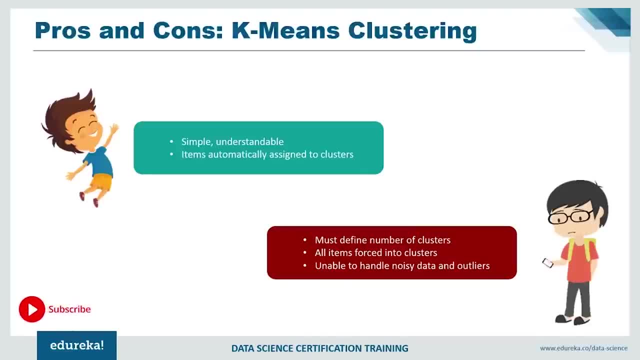 clusters or not being able to guess the correct number of clusters. so, and most of all, it's unable to handle the noisy data and the outliners, because, anyways, machine learning engineers and data scientists have to clean the data. but then again it comes down to the analysis, what they are doing and the method that. 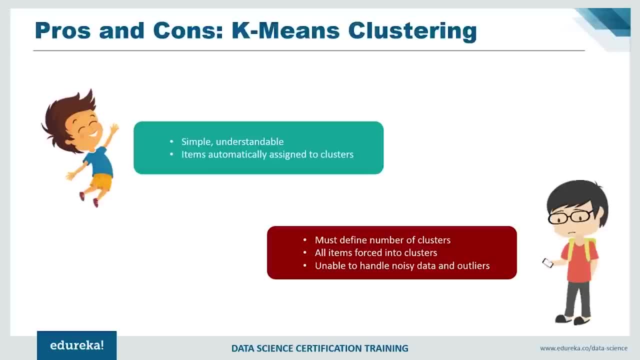 they are using. so typically people do not clean the data for k-means clustering. or even if they clean, there are- sometimes there are now- see noisy and outliners- data like the whole model. so that was all for k-means clustering. so what we're? 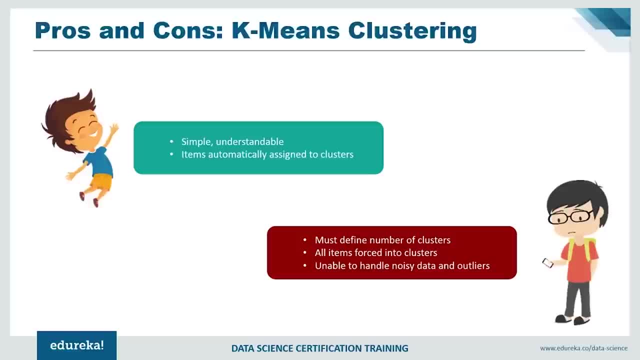 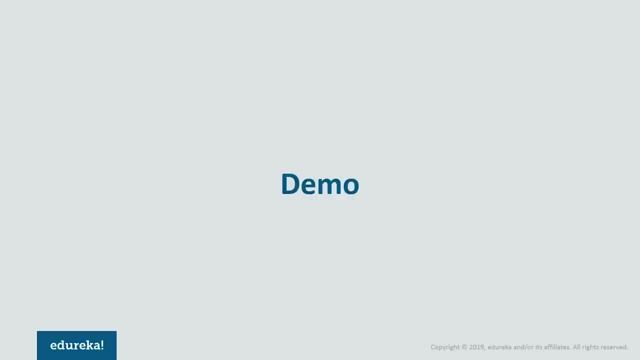 gonna do is now use k-means clustering for the movie data set. so we have to find out the number of clusters and divide it accordingly. so the use case is that first of all, we have a data set of 5,000 movies and what we want to do is: 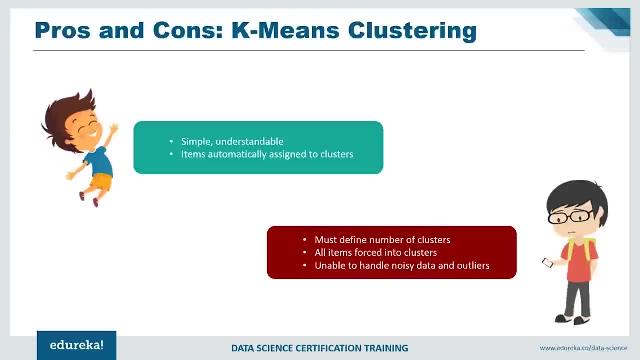 Now, K-Means is not exactly a very good method. So let's understand the problem. What are the pros and cons of K-Means clustering? We know that K-Means is simple and understandable. Everyone learns it at the first go. 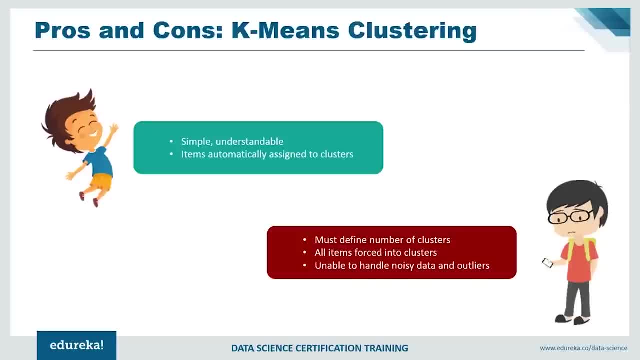 The items automatically assigned to the clusters. Now if we have a look at the cons, so first of all one needs to define the number of clusters. This is a very heavy task, as if we have 3,, 4 or if we have 10 categories. 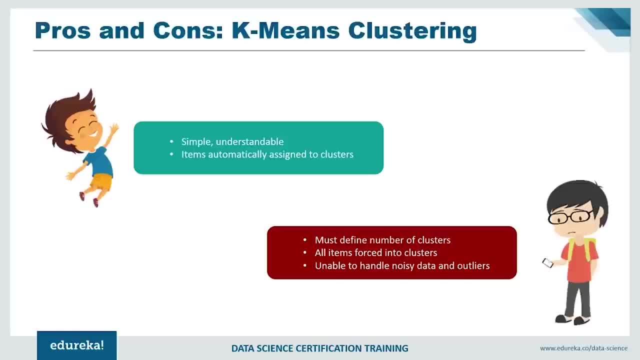 and if we do not know what the number of clusters are going to be, it's very difficult for anyone to you know to guess the number of clusters. Now, all the items are forced into the clusters, So whether they are actually belong to any other cluster or any other, 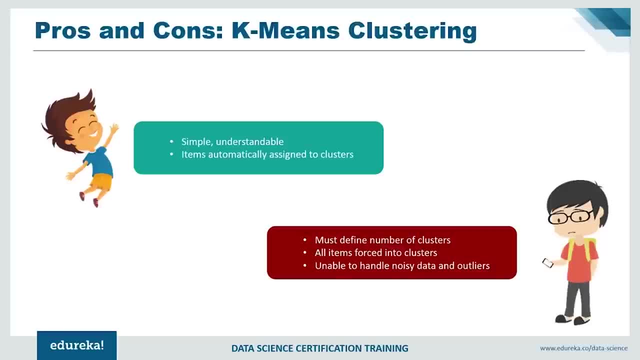 category, they are forced to lie in that other category in which they are closest to. Now this again happens because of the number of clusters, with not defining the correct number of clusters or not being able to guess the correct number of clusters. So, and most of all, it's unable to handle the noisy data and the 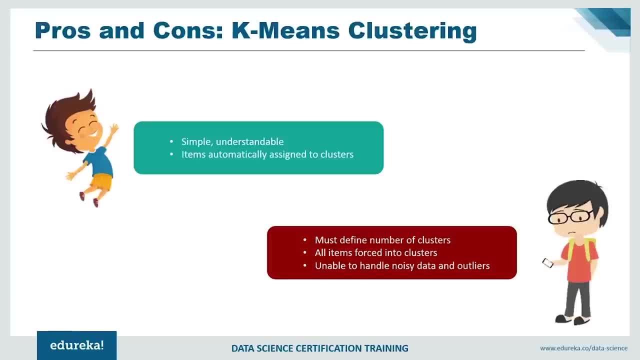 outliners because, anyways, machine learning engineers and data scientists have to clean the data. But then again it comes down to The analysis, what they are doing and the method that they are using. So typically people do not clean the data, for k-means clustering or even 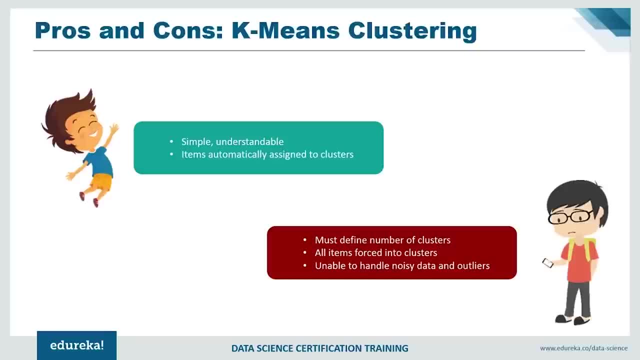 if they clean there are. sometimes there are noisy, noisy and outliners data which affect the whole model. So that was all for k-means clustering. So what we're going to do is now use k-means clustering for the movie data set. 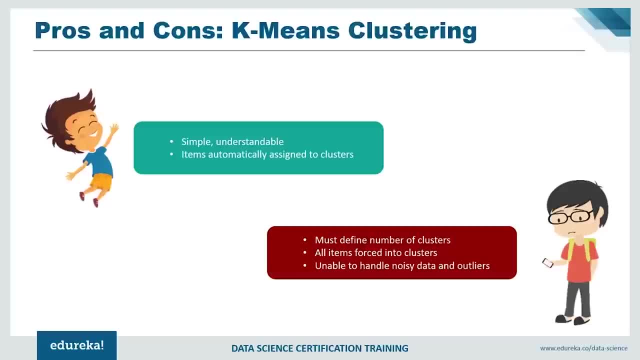 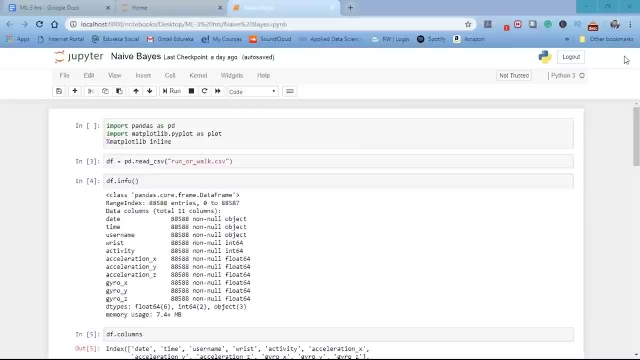 So we have to find out the number of clusters and divide it accordingly. So they use Is that, first of all, we have a data set of 5,000 movies and what we want to do is group them, with the movies, into clusters based on the. 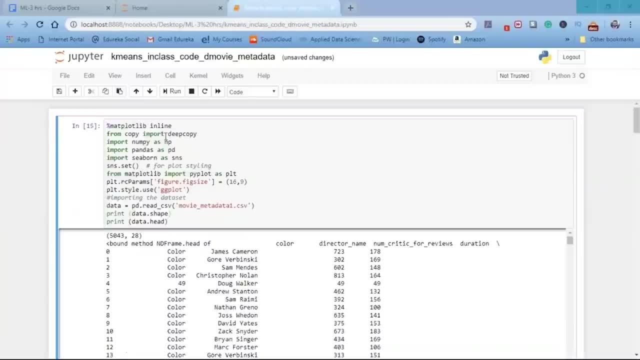 Facebook likes. So, guys, let's have a look at the demo here. So, first of all, what we're going to do is import deep copy- numpy, Panda, Seaborn, the various libraries which we're going to use now- and from my product. 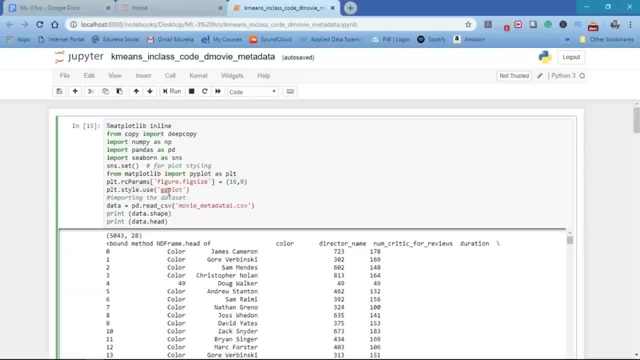 We're going to use fly by plot and we're going to use as ggplot. and next, What we're going to do is import The data set and look at the shape of the data set. So if you have a look at the shape of the data set, we can see that it. 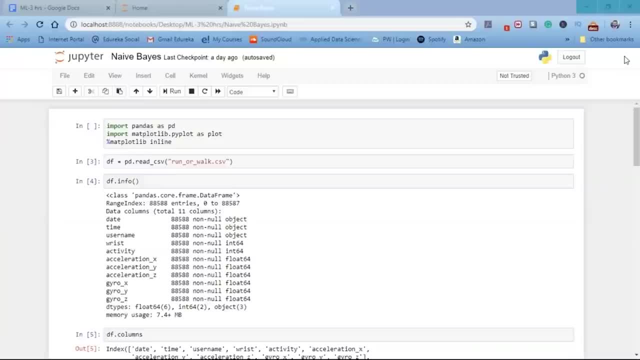 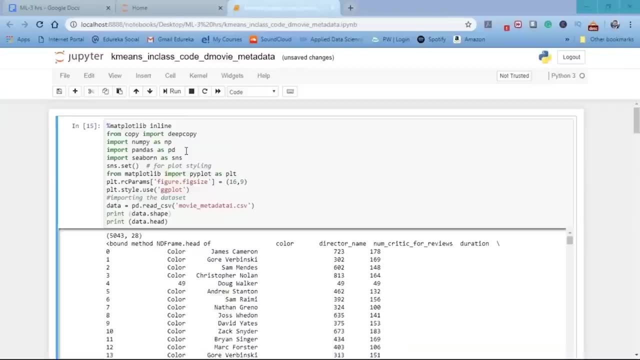 group them with the movies into clusters based on the Facebook likes. so, guys, let's have a look at the demo here. so, first of all, what we're going to do is import deep copy, numpy, pandas, seaborn, the various libraries which we're going to use now, and from matplotlib we're going to use fly by plot and we're going to use 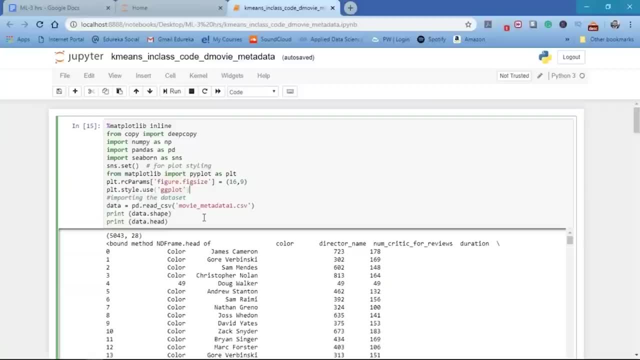 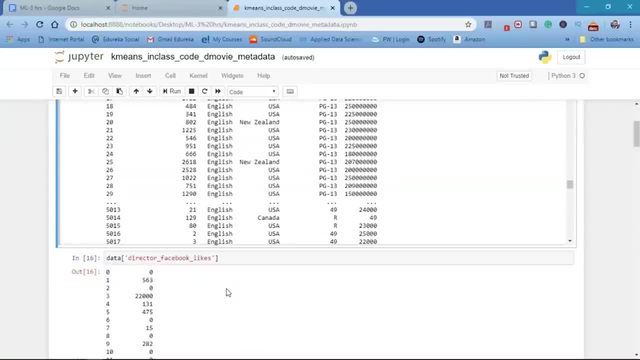 this ggplot and next, what we're going to do is import the data set and look at the shape of the data set. so if you have a look at the shape of the data set, we can see that it has 5,043 rows with 28 columns. and if you have a look at the 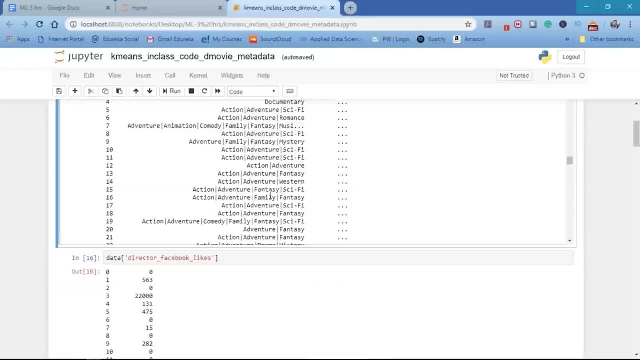 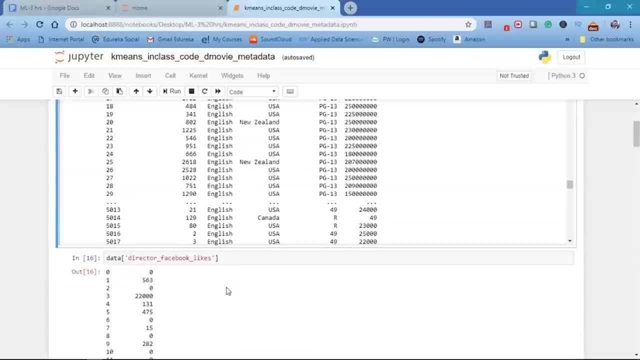 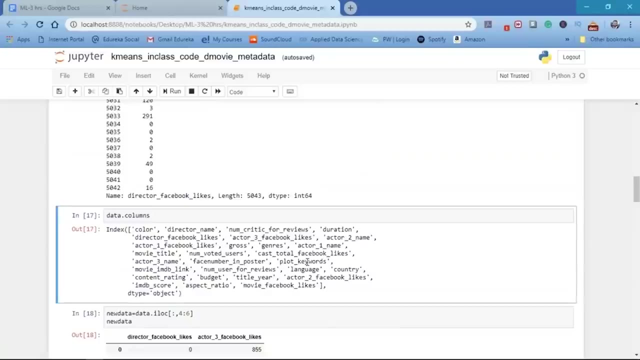 head of the data set, we can see it has 5,043 data points. so what we're going to do is place the data points in the plot. we take the director Facebook likes and we have a look at the data columns. yeah, face number in poster cast total Facebook likes, director. 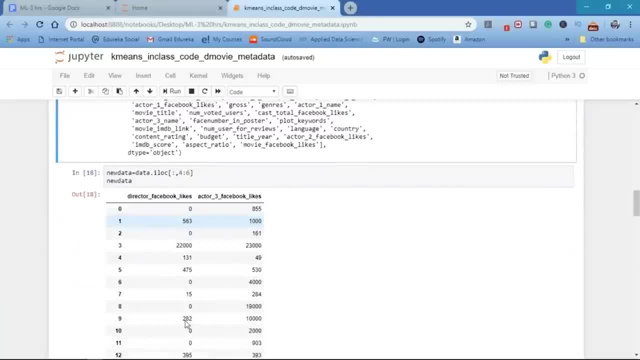 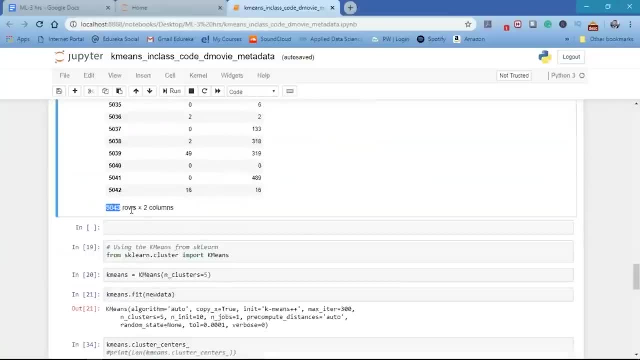 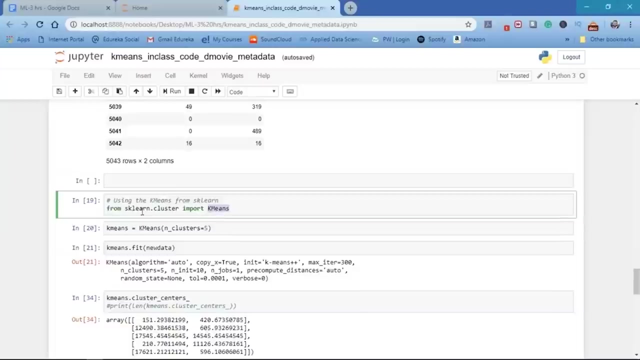 Facebook likes. so what we have done here now is taking that a director- Facebook likes and the actor 3 Facebook likes, right? so we have five thousand forty three rows and two columns now using the k-means from escalator. what we're going to do is import it. first, we're going to import k-means from sklearncluster. 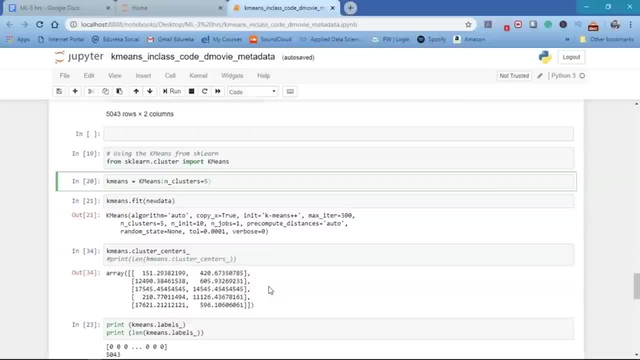 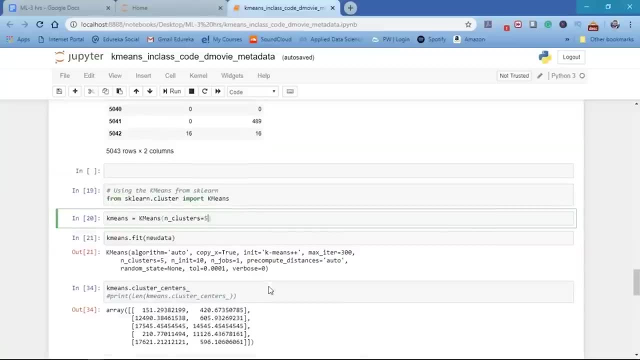 remember, guys, sklearn is a very important library in python for machine learning. so, and the number of cluster, what we're going to do is provide as five. now this again: the number of cluster depends upon the sse, which is the sum squared errors or the. we're going to use the 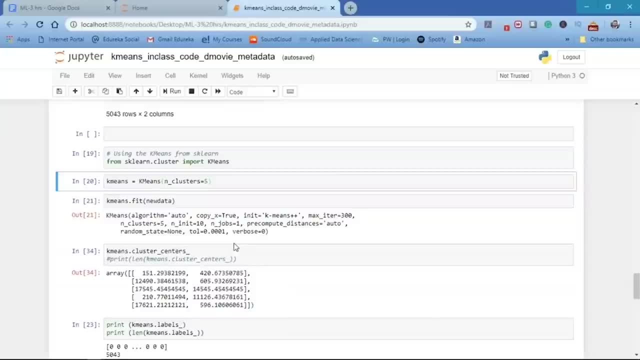 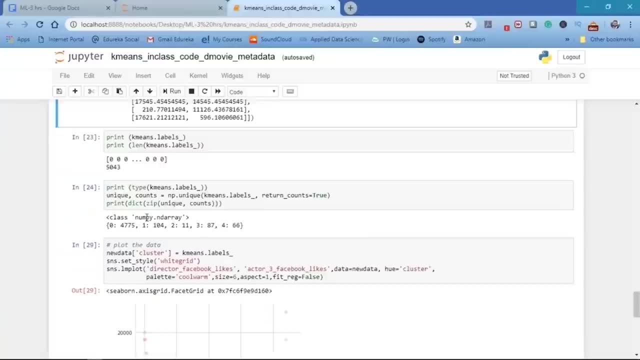 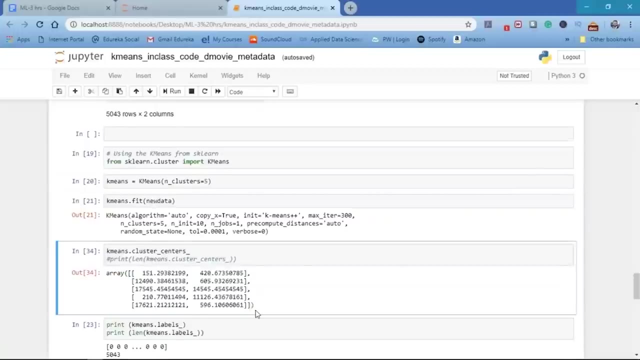 l1 method. so i'm not going to go into the details of that again. so we're going to fit the data into the k-meansfit and if we find the cluster centers then for the k-means and print it. so what we find is is an array of five clusters and if we print the label of the k-means cluster. 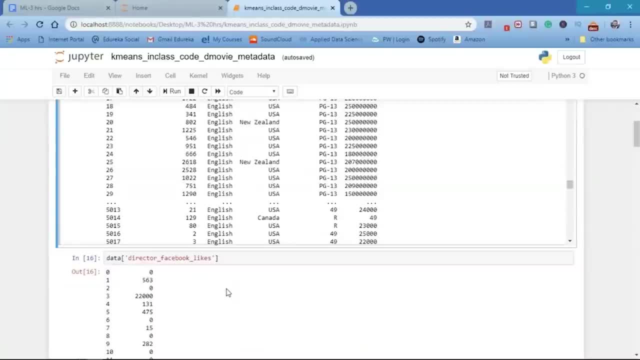 has 5,043 rows with 28 columns And if you have a look at the head of the data set, we can see it has 5,043 data points. So what we're going to do is place the data points in the plot. 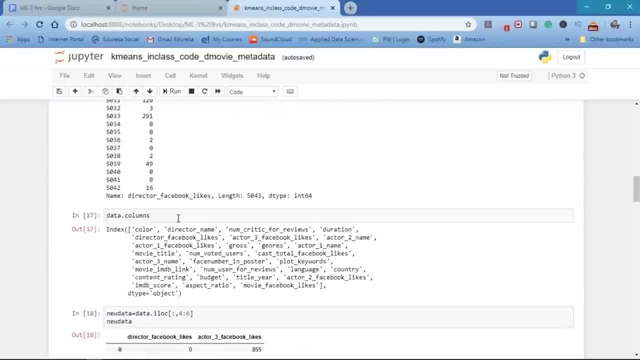 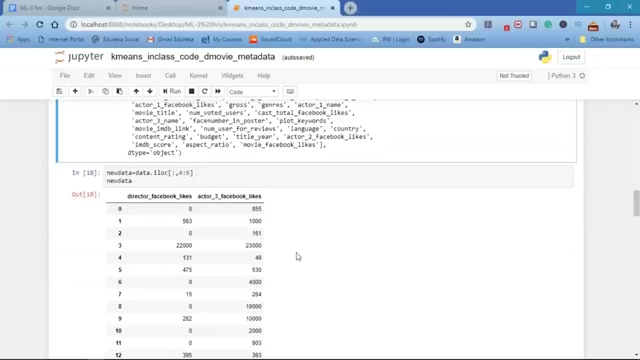 We take the director Facebook likes and we have a look at the data columns. Yeah, face number in poster cast total Facebook likes. Director Facebook likes. So what we have done here now is taking the director Facebook likes and the actor three Facebook likes. right, 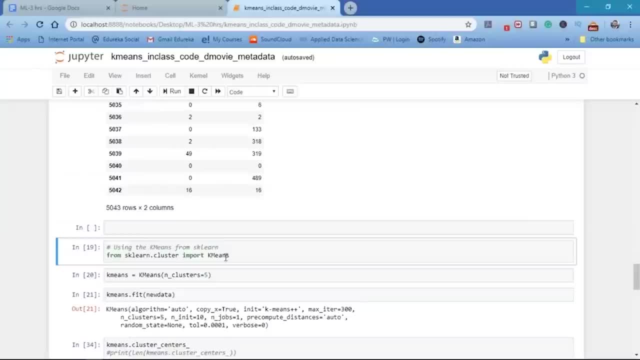 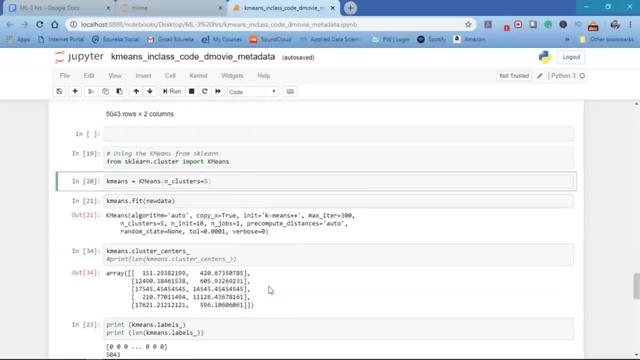 So we have 5,043 rows and two columns Now using the k-means from sklearn. what we're going to do is import it first. We're going to import k-means from sklearncluster. Remember, guys, sklearn is a very important library in python for 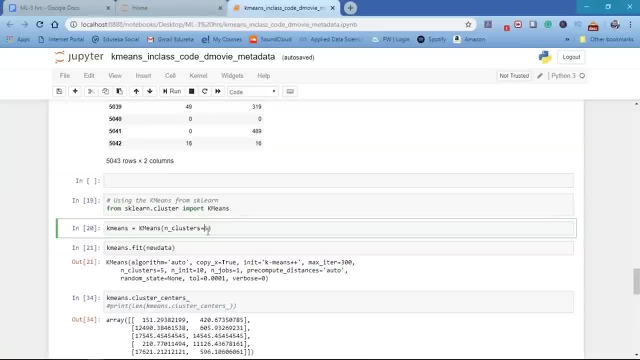 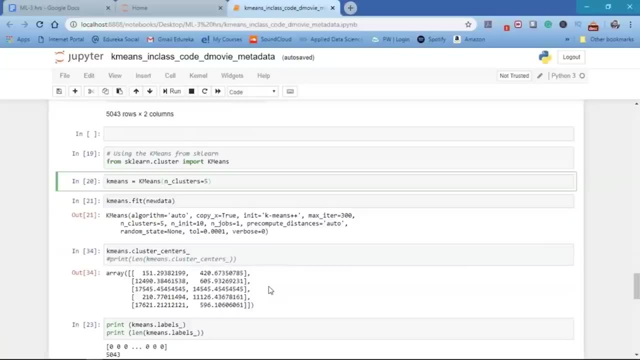 machine learning. So, and the number of cluster? what we're going to do is provide as five. Now this again, the number of cluster depends upon the SSE, which is the sum squared errors or the. we're going to use the elbow method. 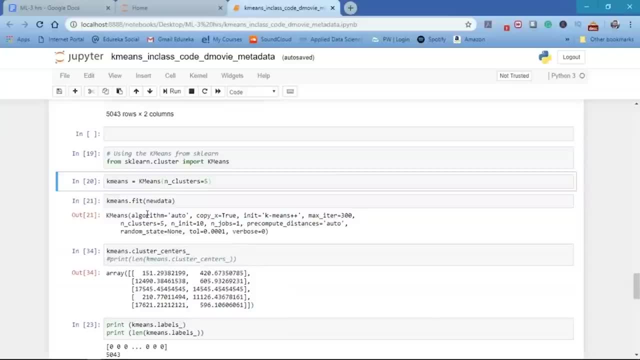 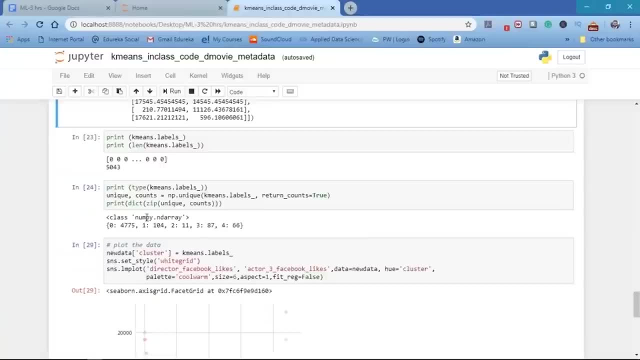 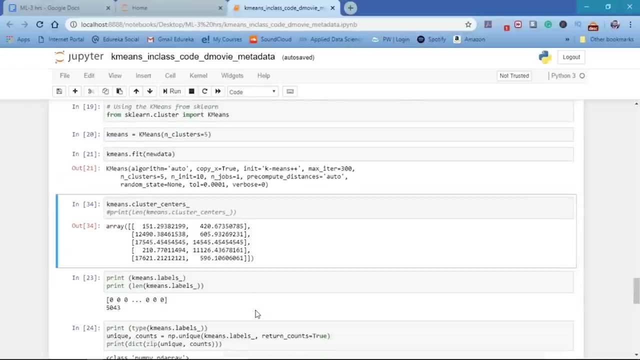 So I'm not going to go into the details of that again. So we're going to fit the data into the k-meansfit and if you find the cluster centers, then for the k-means and print it. So what we find is is an array of five clusters and if we print the 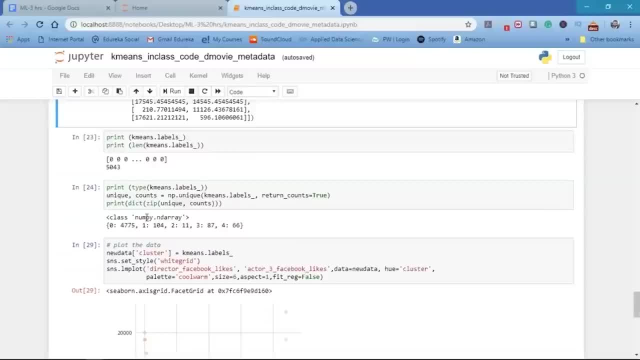 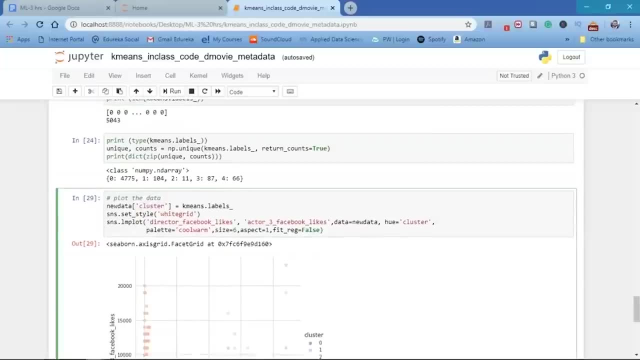 label of the k-means cluster. Now, next, what we're going to do is plot the data which we have with the clusters, with the new data clusters which we have found, and for this we're going to use the seaborn, and, as you can see, here we have 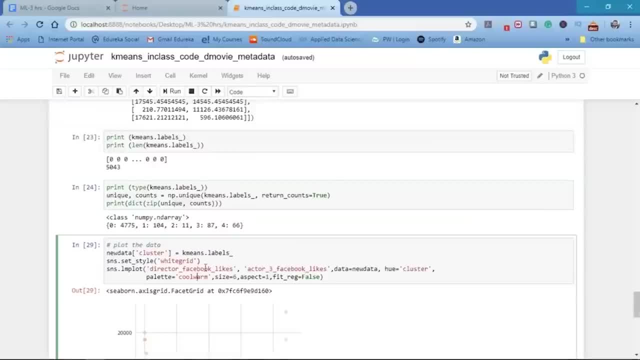 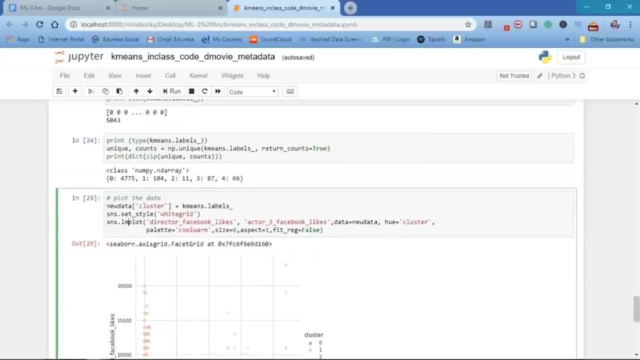 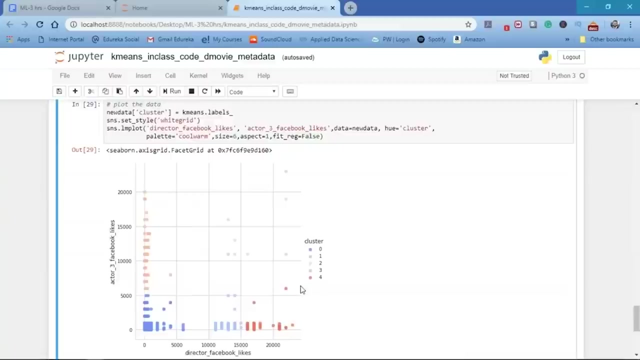 now. next, what we're going to do is plot the data which we have with the clusters, with the new data clusters which we have found, and for this we're going to use the seaborn and, as you can see here, we have plotted the, the data into the grid and you can see here we have five clusters. so probably what i would say is: 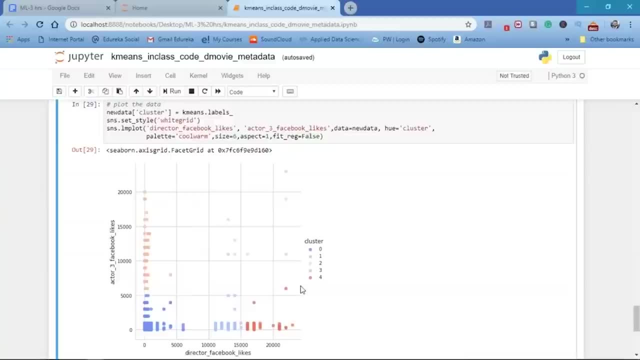 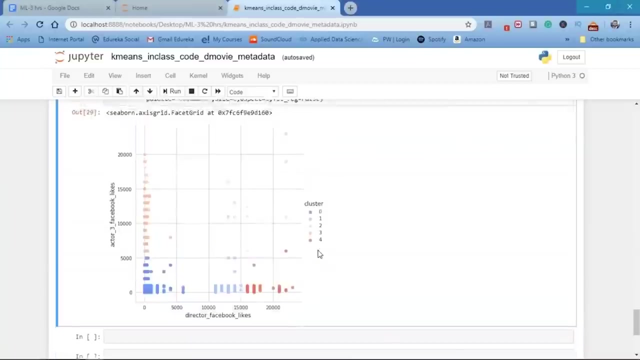 plotted the data into the grid and you can see here We have five clusters. So probably what I would say is that the cluster three and the cluster zero are very, very close, So it might depend. See, that's exactly what I was going to say. is that initially the main? 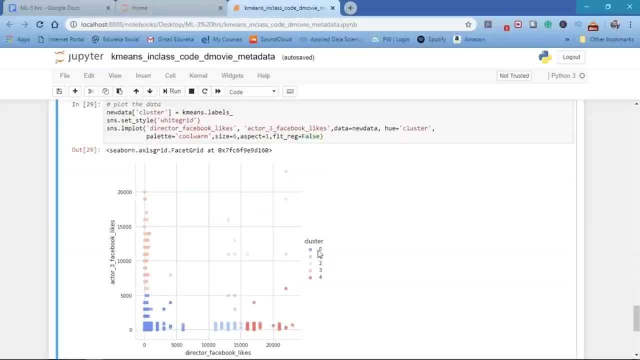 challenge and k-means clustering is to define the number of centers which are the key. So, as you can see here that the third Center and the 0th cluster, the third cluster and the 0th cluster, are very, very close to each other. 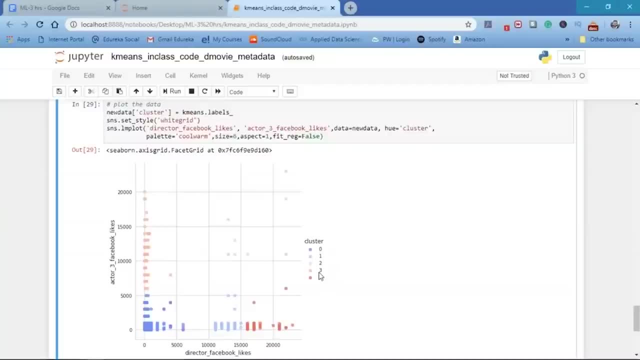 that the cluster three and the cluster zero are very, very close. so it might depend. see, that's exactly what i was going to say is that, initially, the main challenge in k-means clustering is to define the number of centers which are the k. so, as you can see here that the third center and 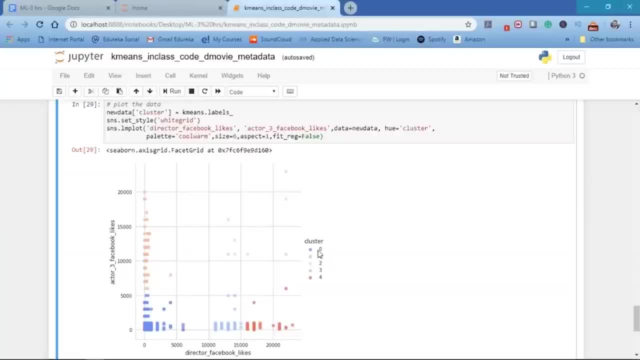 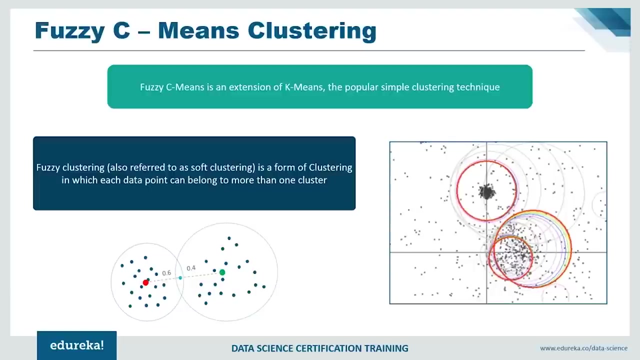 the zeroth cluster, the, the third cluster and the zeroth cluster are very, very close to each other. so, guys, it probably could have been in one another cluster, and the another disadvantage was that we do not exactly know how the points are to be arranged, so it's very difficult to force the data into any other. 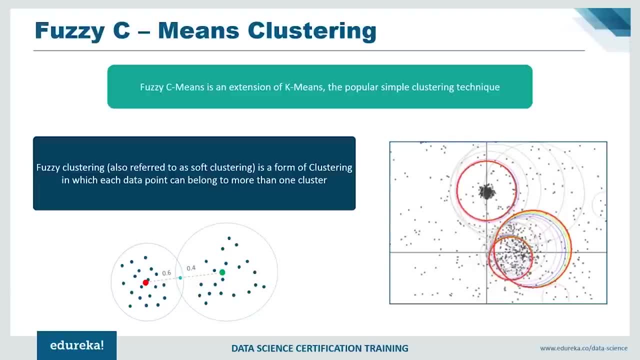 cluster, which makes our analysis a little different, works fine, but sometimes it might be difficult to code in the k-means clustering. now let's understand what exactly is c-means clustering. so the fuzzy c-means is an extension of the k-means clustering, the popular simple clustering technique. 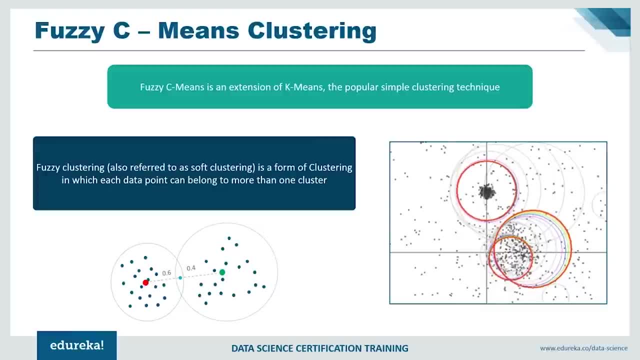 so fuzzy clustering, also referred as soft clustering, is a form of clustering in which each data point can belong to more than one cluster. so k-means tries to find the hard clusters where each one belongs to one cluster, whereas the fuzzy c-means discovers the soft clusters in a. 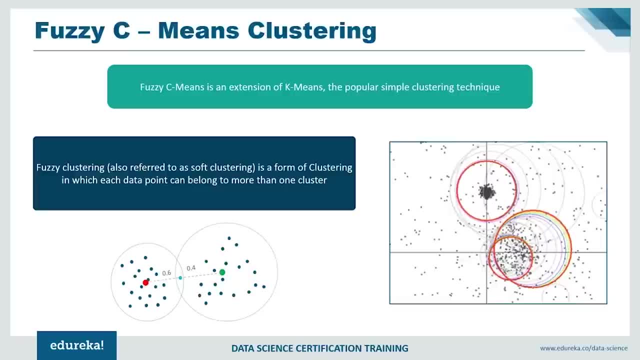 soft cluster. any point can belong to more than one cluster at a time with a certain affinity value to a specific angle. so if we fix that the friendship installs may as well enrich the cuz each. so this is a function where each cluster can have a different Go to a given place from one different. 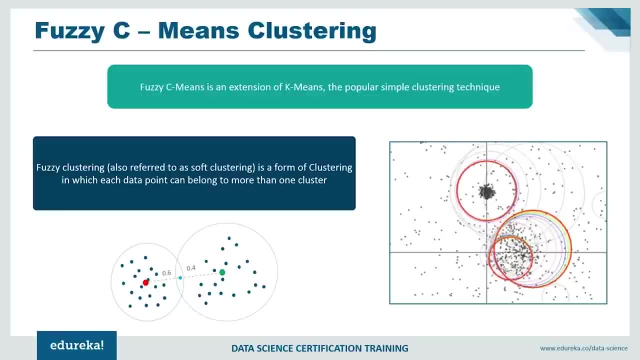 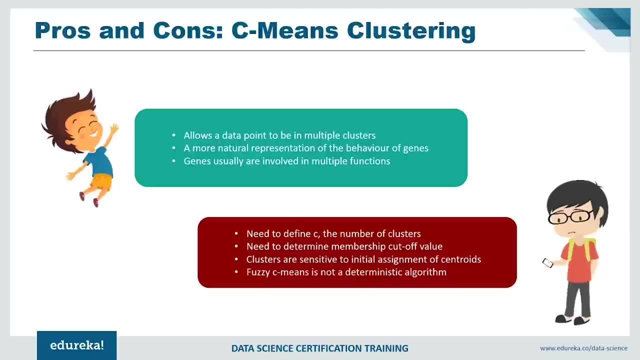 cluster. so inside this bind array we can see the idea that all five cluster are in one space. so you can go from всегда to give me a specific name, and then it lifetime. God, insane, let's again. we're approaching each cup or whatever you can say. ie a cluster which is long, it dobbing is. 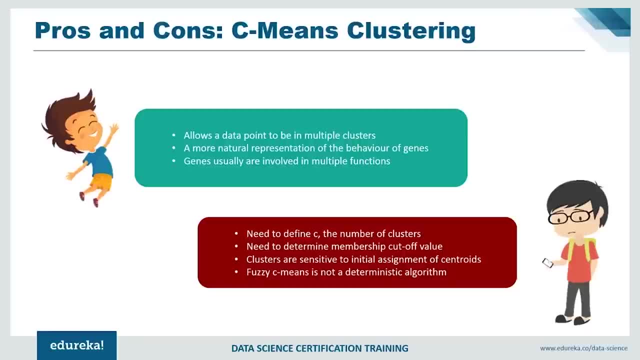 means so, and and this affinity is proportional to the distance from the point to the centroid of the cluster. now, then again, we have the pros and cons of fuzzy. c means so: first of all, it allows a data point to be in multiple clusters. that's a pro. it's a more neutral representation of the behavior of 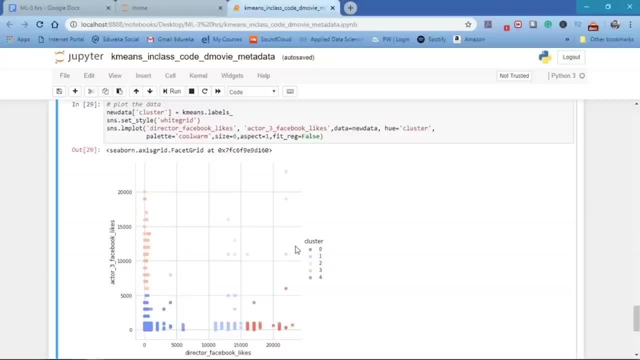 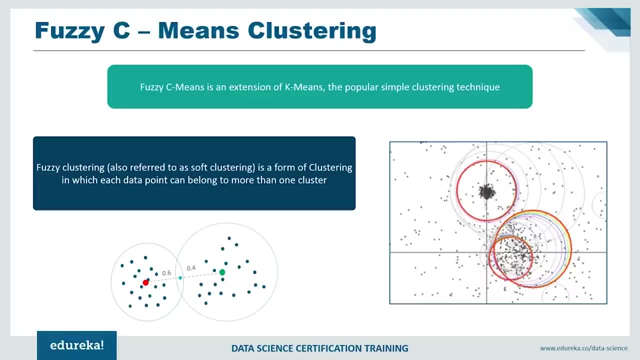 So, guys, it probably could have been in one another cluster, and the another disadvantage was that we do not exactly know how the points are to be arranged, So it's very difficult to force the data into any other. The cluster, which makes our analysis a little different, works fine. 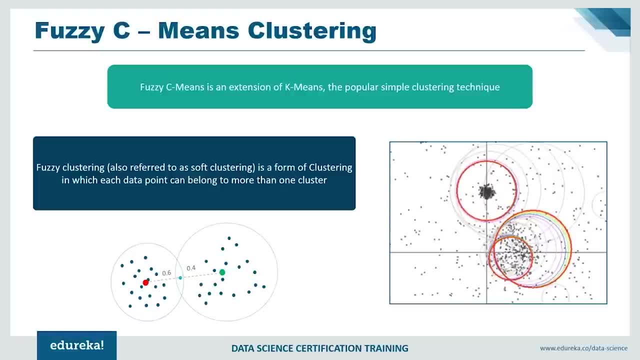 but sometimes it might be difficult to code in the k-means clustering. Now let's understand what exactly is c-means clustering. So the fuzzy c-means is an extension of the k-means clustering, of the popular simple clustering technique. So fuzzy clustering, also referred as soft clustering, is a form of 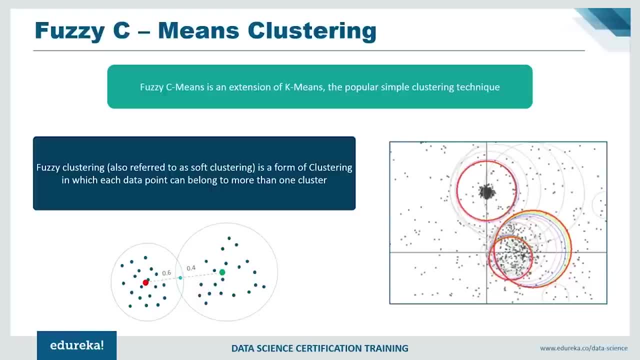 clustering in which each data point can belong to more than one cluster. So k-means tries to find the hard clusters, where each one belongs to one cluster, Whereas the fuzzy c-means discovers the soft clusters. In a soft cluster, any point can belong to more than one cluster at a time, with a certain. 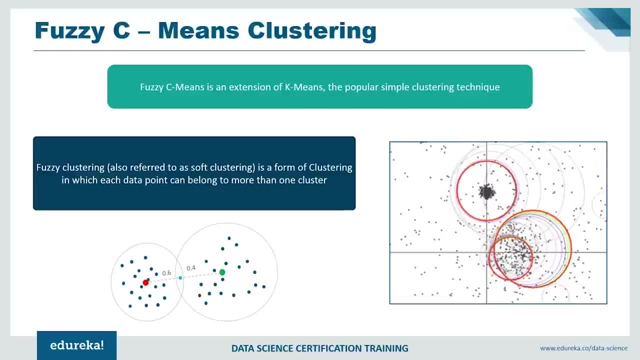 affinity value towards each Fuzzy c-means assigns the degree of membership, which ranges from 0 to 1, to an object to a given cluster. So there is a stipulation that the sum of fuzzy membership of an object to all the cluster. 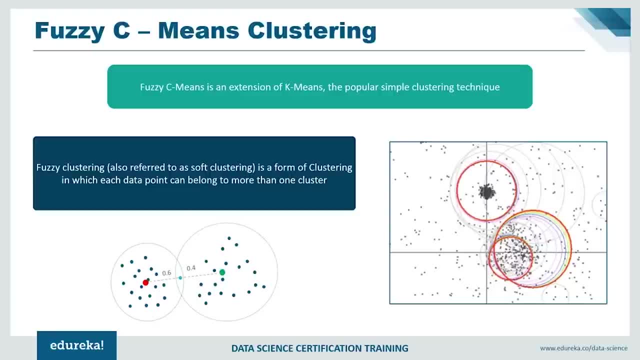 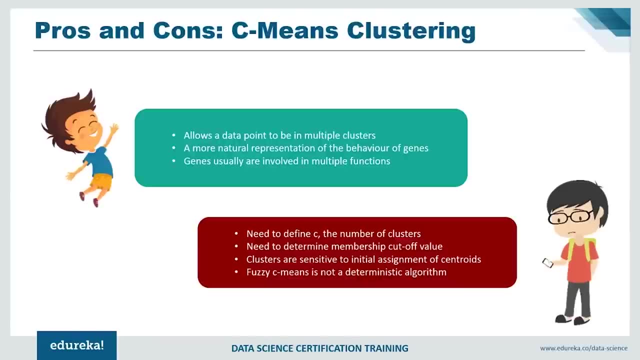 It belongs to must be equal to 1.. So the degree of membership of this particular point to pull of these clusters are 0.6 and 0.4 and if we add up we get 1.. So that is one of the logic behind the fuzzy c-means and this affinity. 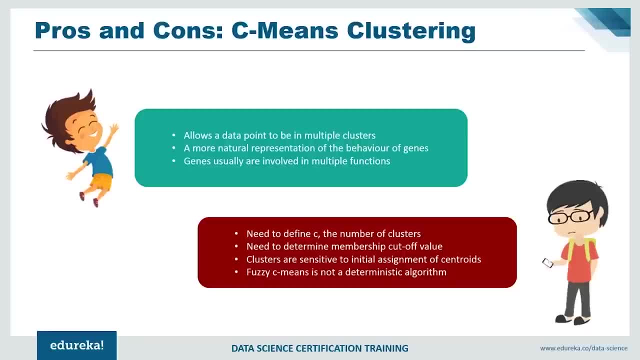 is proportional to the distance from the point to the centroid of the cluster. Now then again, we have the pros and cons of fuzzy c-means. So, first of all, it allows a data point to be in multiple clusters. That's a pro. 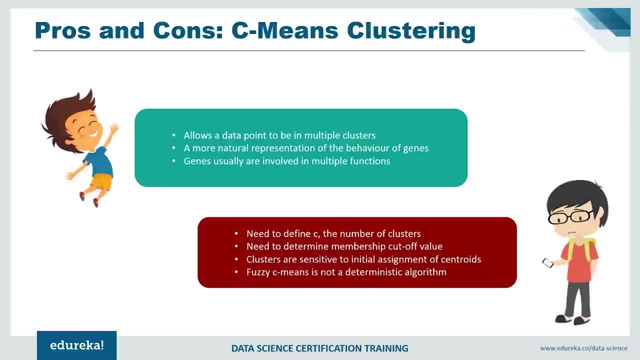 It's a more neutral representation of the behavior of genes. Genes usually are involved in multiple functions, So it is a very good type of clustering. when we're talking about genes First of all and again, if we talk about the cons, again we have to 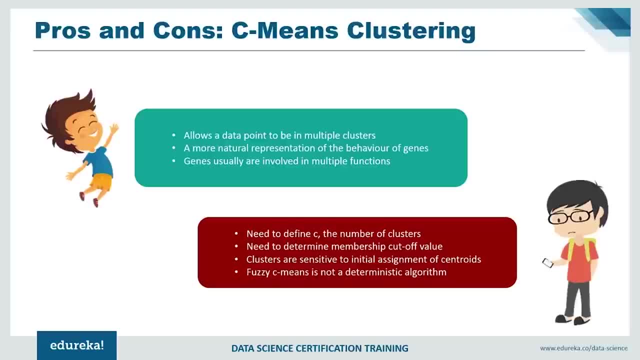 define c, which is the number of clusters, same as k. Next we need to determine the membership cutoff value also. So that takes a lot of time and it's time-consuming, and the clusters are sensitive to initial assignment of centroid. so a slight change or deviation. 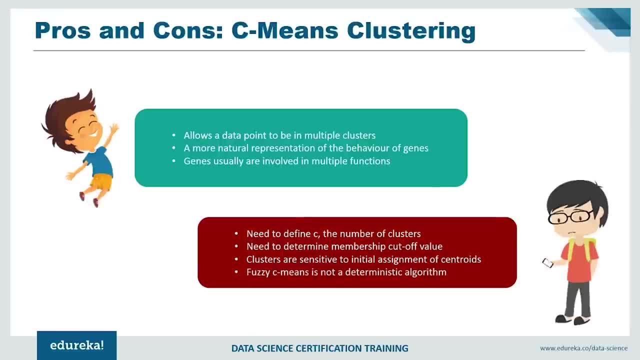 genes. genes usually are involved in multiple functions, so it is a very good type of clustering. when we are talking about genes, first of and again if we talk about the cons, again we have to define c, which is the number of clusters same as k. next we need to determine the membership cutoff value. 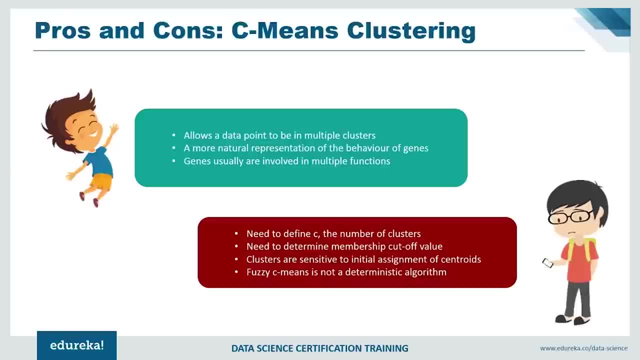 also so that takes a lot of time and it's time consuming and the clusters are sensitive to initial assignment of centroid. so a slight change or a deviation from the centroid is going to result in a very different kind of- you know a funny kind of output we get from the fuzzy c means. 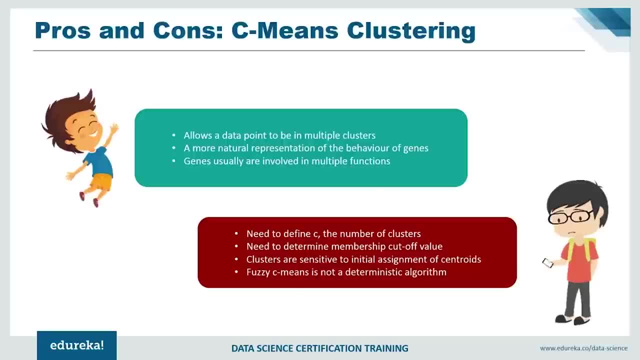 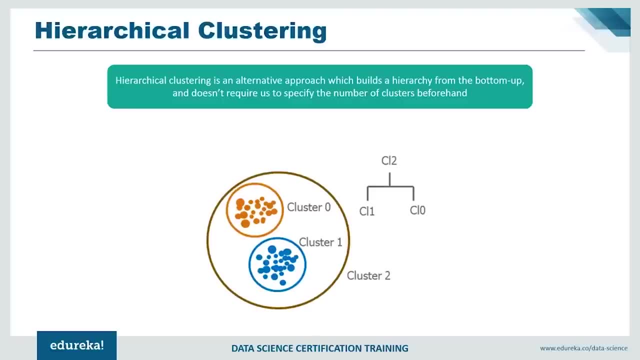 and one of the major disadvantage of c means clustering is that it's this, this, this, the non-deterministic algorithm, so it does not give you a particular output, as in such that's that. now let's have a look at the third type of clustering, which is the hierarchical clustering. 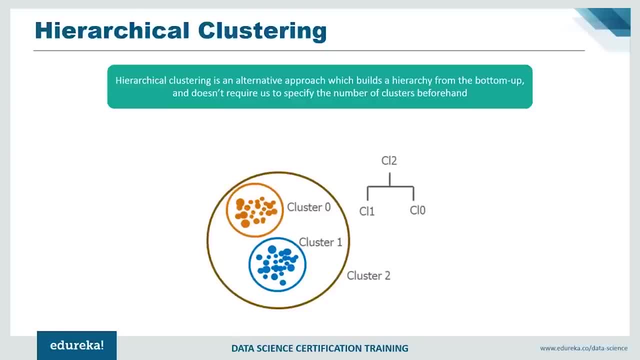 so a hierarchical clustering is an alternative approach which builds a hierarchy from the bottom up or the top to bottom and does not require to specify the number of clusters beforehand. now the algorithm works as in: first of all, we put each data point in its own cluster and if either closes to cluster and 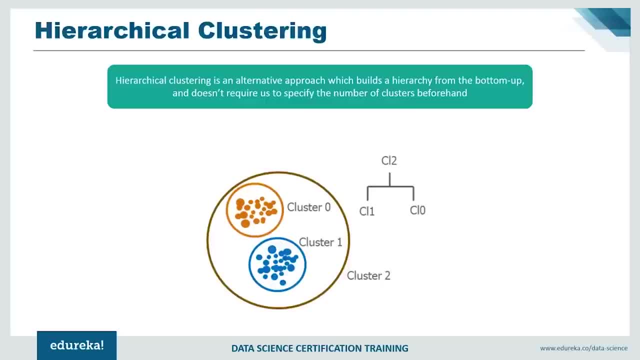 combine them into one more cluster. repeat the above step till the data points are in a single cluster. now there are two types of hierarchy clustering: one is agglomerative clustering and the other one is division clustering. so agglomerative clustering builds the dendrogram from bottom level, while the 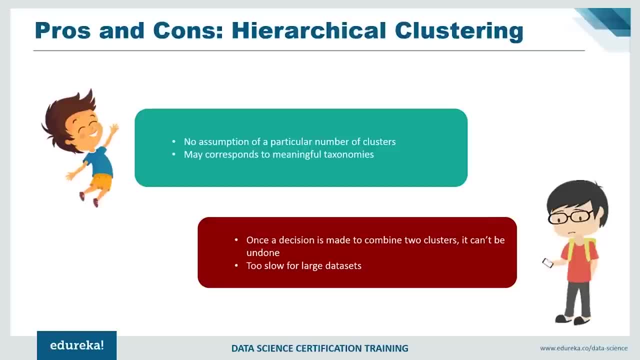 division clustering. it starts all the data points in one cluster, the root cluster. now again, hierarchical clustering also has some sort of pros and cons. so in the pros, though, no assumption of a particular number of clusters is required to build a dendrogram from the bottom level, while the division clustering 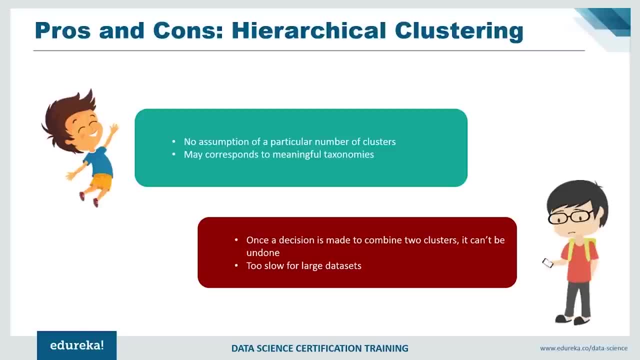 is required and it may correspond to meaningful taxonomies, whereas if we talk about the cons, once a decision is made to combine two clusters, it cannot be undone, and one of the major disadvantage of these hierarchical clustering is that it becomes very slow if we talk about very, very 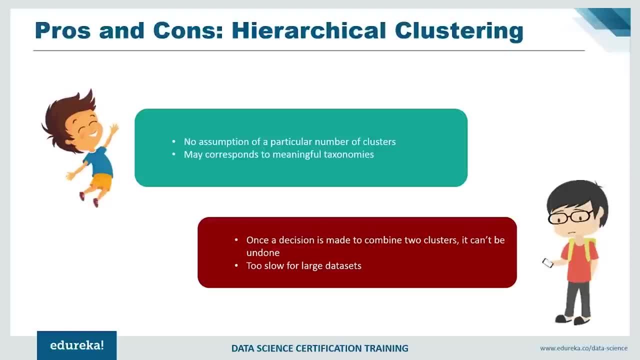 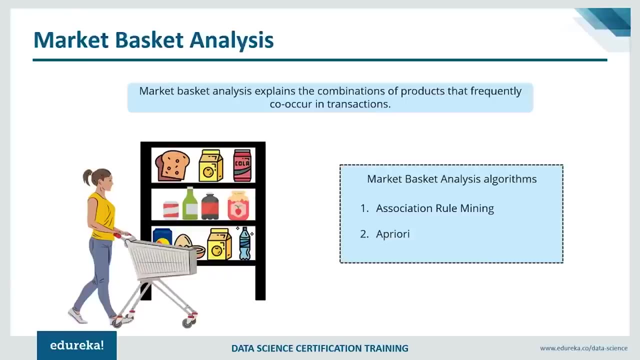 large data sets and nowadays i think every industry are using large data sets and collecting large amounts of data. so hierarchical clustering is not the apt or the best method someone might use. so there's that now when we talk about unsupervised learning. so we have k-means clustering. 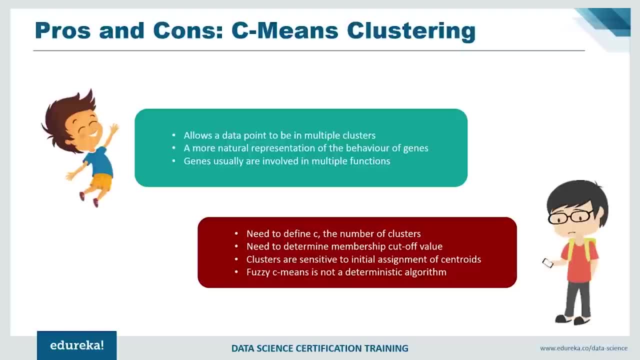 from the centroid is going to result in a very different kind of- you know a funny kind of output we get from the fuzzy c-means, And one of the major disadvantages of c-means clustering is that it's there's a non-deterministic algorithm. 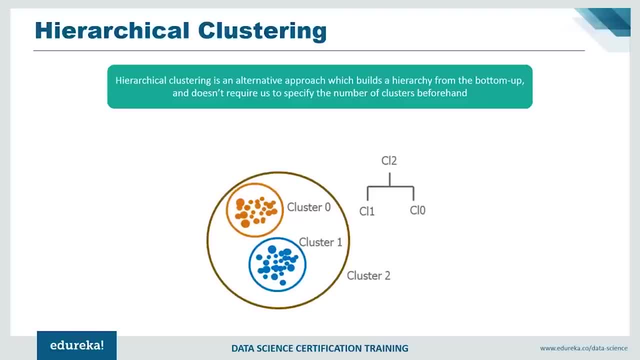 So it does not give you a particular output as in such. that's that. Now let's have a look at the third type of clustering, which is the hierarchical clustering. So a hierarchical clustering is an alternative approach which builds a hierarchy from the bottom up. 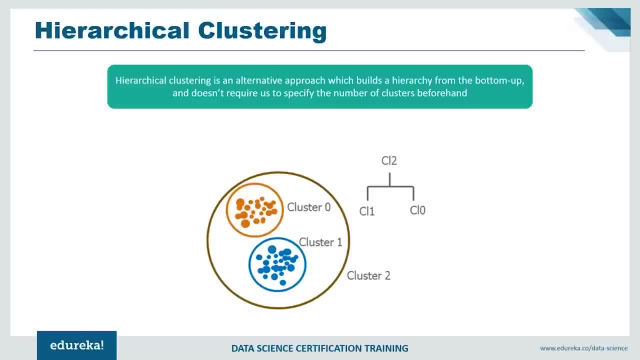 Or the top to bottom, and does not require to specify the number of clusters beforehand. Now the algorithm works as in: first of all, we put each data point in its own cluster, identify the closest to cluster and combine them into one more cluster. 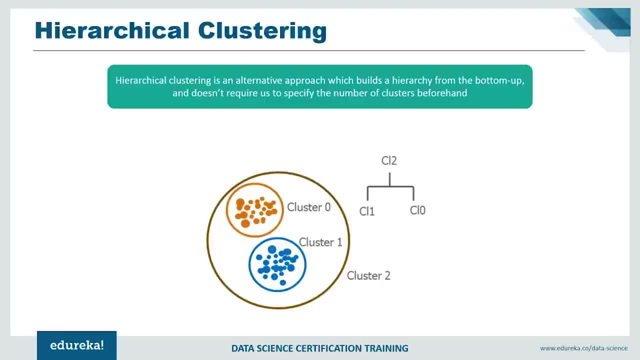 Repeat the above step till the data points are in a single cluster. Now there are two types of hierarchy clustering. One is agglomerative clustering and the other one is division clustering. So agglomerative clustering builds the dendrogram from bottom level, while the division clustering 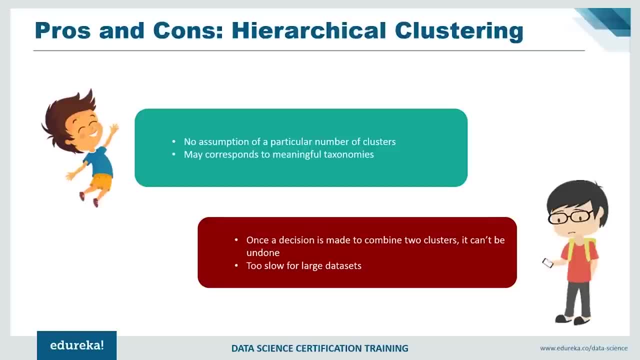 Starts all the data points in one cluster, the root cluster. Now again, hierarchical clustering also has some sort of pros and cons. So in the pros, though, no assumption of a particular number of cluster is required and it may correspond to meaningful taxonomies. 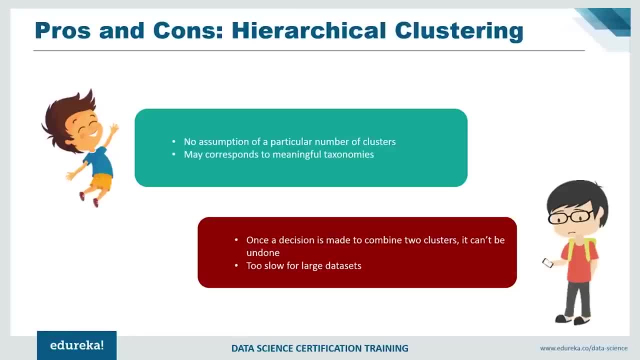 Whereas if we talk about the cons, once a decision is made to combine two clusters, it cannot be undone, and one of the major disadvantage of these hierarchical clustering is that it becomes very slow if we talk about very, very large data sets, And nowadays I think every industry are using large data sets and collecting. 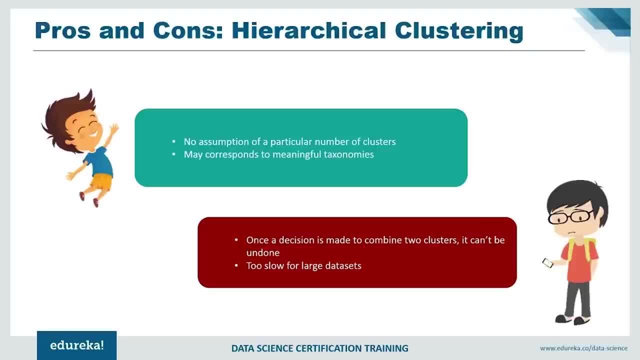 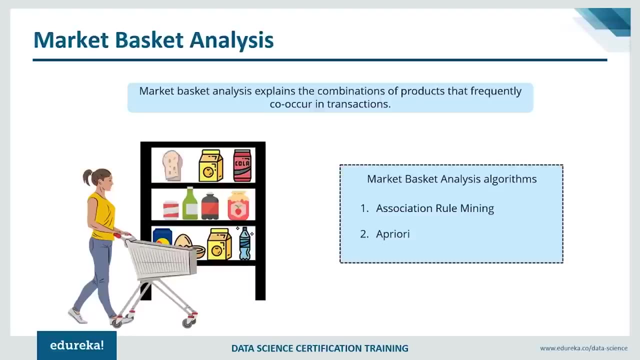 large amounts of data. So hierarchical clustering is not the apt or the best method someone might need to go for. So there's that Now, when we talk about unsupervised learning, so we have key means, clustering. and again there's another important term which people usually 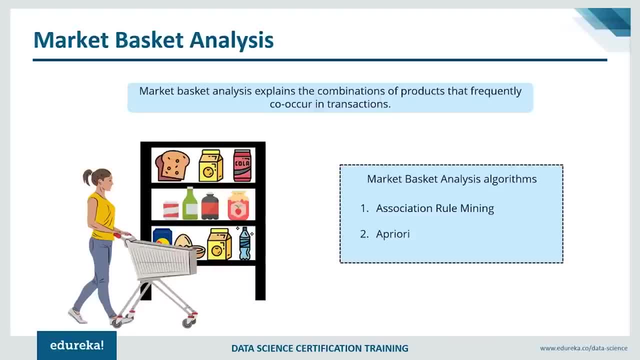 miss while talking about unsupervised learning. and there's one very important concept of market basket analysis. Now it is one of the key techniques used by large retailers to uncover association between items. Now it works by looking for combination of items that occur together. 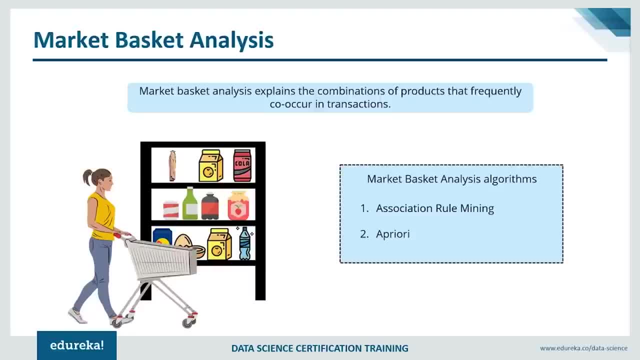 and again. there's another important term which people usually miss while talking about unsupervised learning, and there's one very important concept of market basket analysis. now it is one of the key techniques used by large retailers to uncover association between items. now it works by looking. 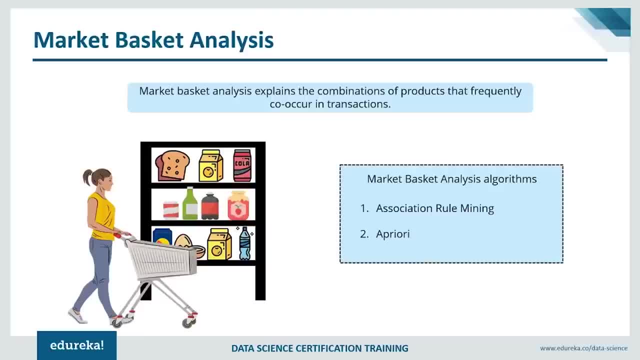 for a combination of items that occur together frequently in the transaction, and it's a very useful way to identify the relationships between the items that the people buy. for example, people who buy bread also tend to buy butter. the marketing team at the retail stores should target customers. 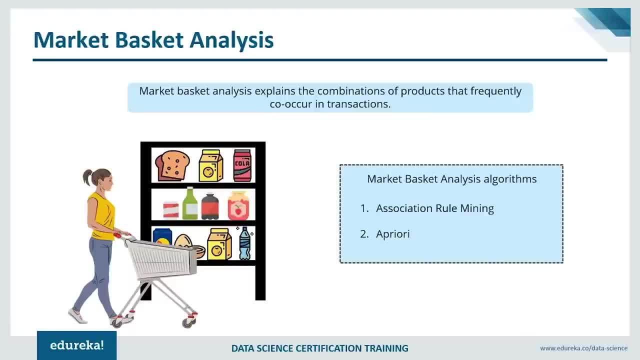 who buy bread and butter and provide them an offer so that they buy a third item like an egg. so if a customer buys bread and butter and sees a discount or an offer on eggs, he will be encouraged to spend more money and buy the eggs. now, this is what market basket analysis is all about, so let's 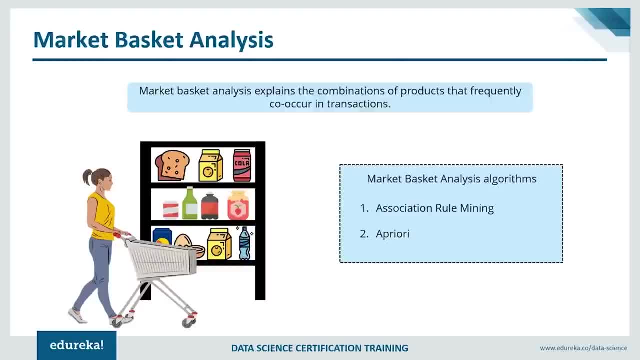 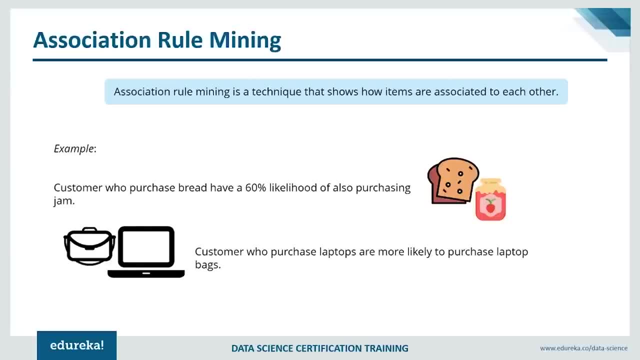 now to find the association between the two items and make predictions about what the customers will buy. there are two algorithms, which are the association rule mining and the a priori algorithms. so let's discuss each of these algorithms with an example. first of all, if we have a look at the 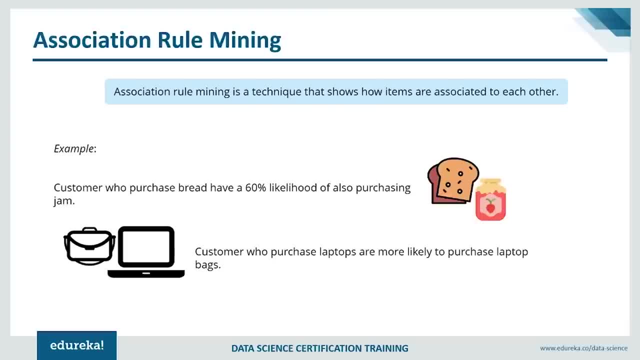 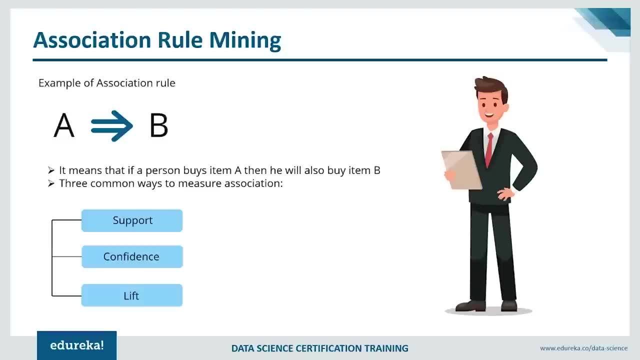 association rule mining. now it's a technique that shows how items are associated to each other. for example, customers who purchase bread have a 60 percent likelihood of also purchasing jam, and customers who purchase bread have a 60 percent likelihood of also purchasing jam. and customers- customers who purchase laptop are more likely to purchase laptop bags. now, if you take an example of 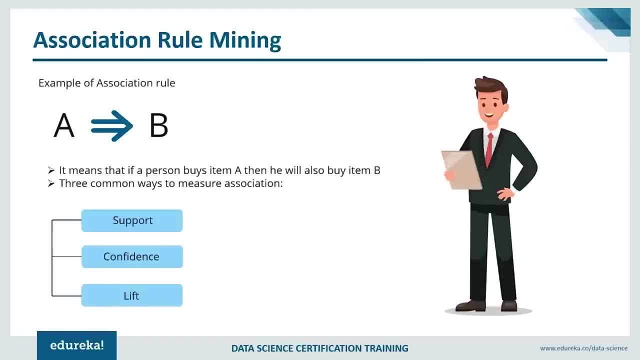 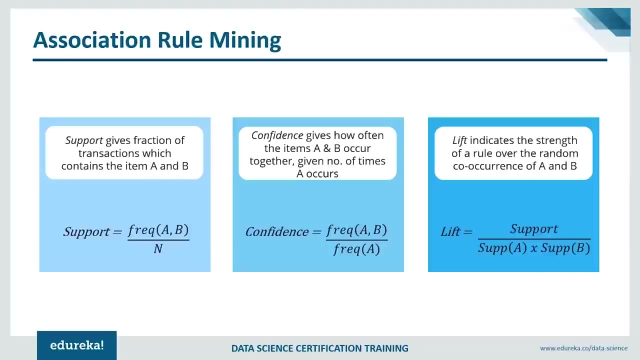 an association rule. if we have a look at the example here, a arrow b. it means that if a person buys an item a, then he will also buy an item b. now there are three common ways to measure a particular association, because we have to find these rules on the basis of some statistics, right? so what we do? 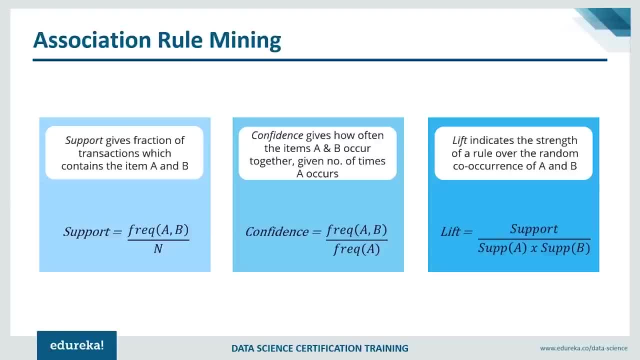 is: use, support, confidence and lift now these three common ways and the measures to have a look at the associated rule mining and know exactly how good is that rule. so first of all, we have support. so support gives the fraction of the transaction which contains an item a and b, so it's basically 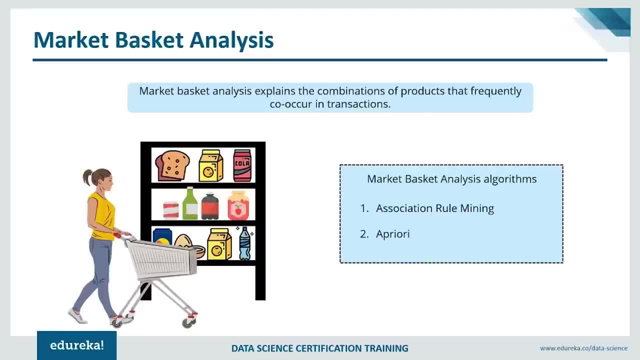 frequently in the transactions. To put it another way, it allows retailers to identify the relationships between the items that the people buy. For example, people who buy bread also tend to buy butter. The marketing team at the retail stores should target customers who buy bread and butter. 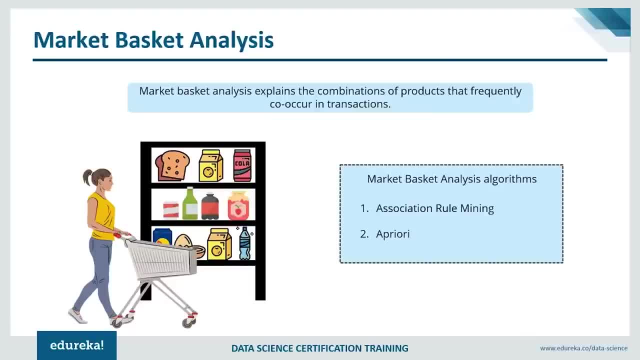 and provide them an offer So that they buy a third item like an egg. So if a customer buys bread and butter and sees a discount or an offer on eggs, he will be encouraged to spend more money and buy the eggs. Now, this is what market basket analysis is all about. 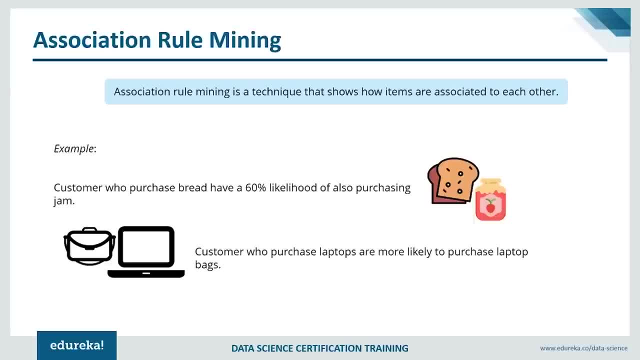 Now to find the association between the two items and make predictions about what the customers will buy. There are two algorithms, which are the association rule mining and the a priori algorithms. So let's discuss each of these algorithm with an example. First of all, if we have a look at 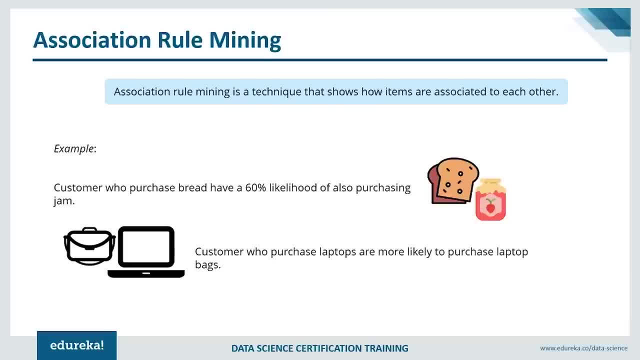 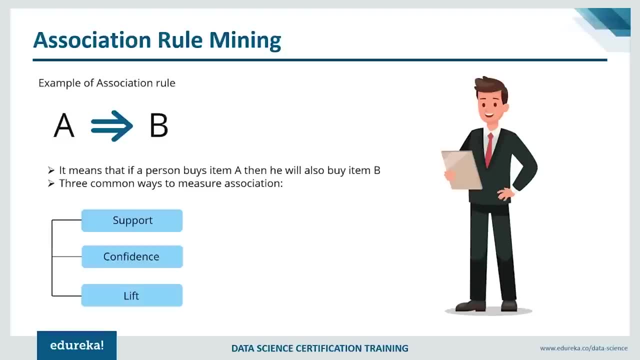 The association rule mining. Now it's a technique that shows how items are associated to each other. For example, customers who purchase bread have a 60% likelihood of also purchasing jam, and customers who purchase laptop are more likely to purchase laptop bags. 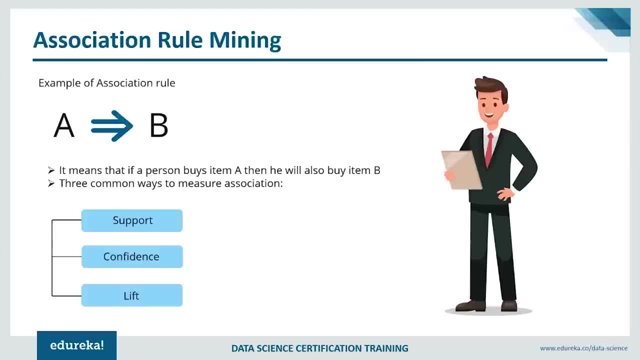 Now, if you take an example of an association rule, if you have a look at the example here, A arrow B, it means that if a person buys an atom A, then he will also buy an atom B. Now there are three common ways to measure a particular association. 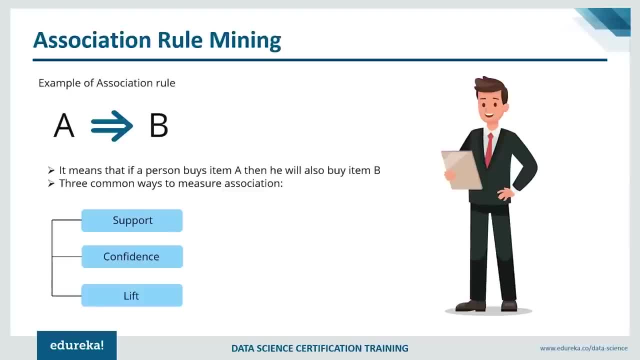 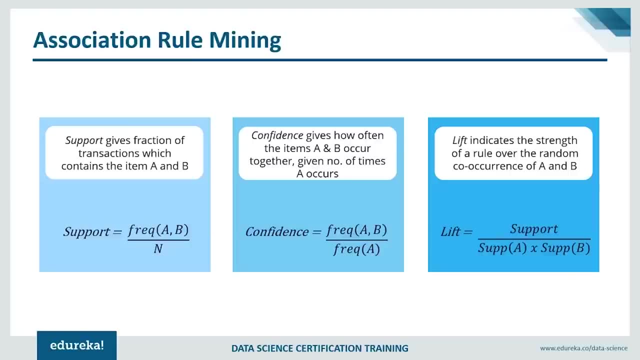 Because we have to find these rules on the basis of some statistics right. So what we do is use, support, confidence and lift Now these three common ways and the measures to have a look at the association rule mining and know exactly how good is that rule. 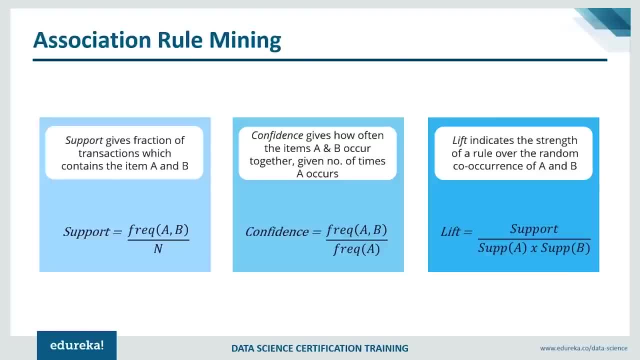 So first of all we have support. So support gives the fraction of the transaction which contains an item A and B, So it's basically the frequency of the item in the whole item set, Whereas confidence gives how often the item A and B. 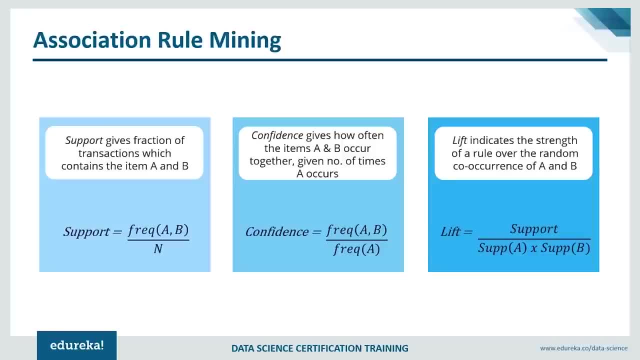 Occurred together, given the number of item, given the number of times A occur. So it's frequency A comma B divided by the frequency of A. Now lift what indicates is the strength of the rule over the random co-occurrence of A and B. 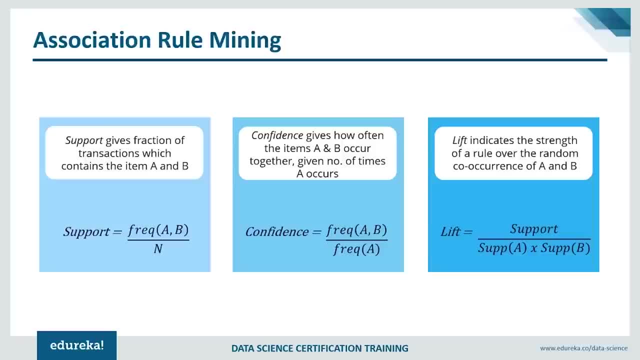 the frequency of the item in the whole item set, whereas confidence gives how often the item a and be awkward together, given the number of item, given the number of times a occur. so its frequency, a comma B, divided by the frequency of a, now left what indicates is the strength of the rule over. 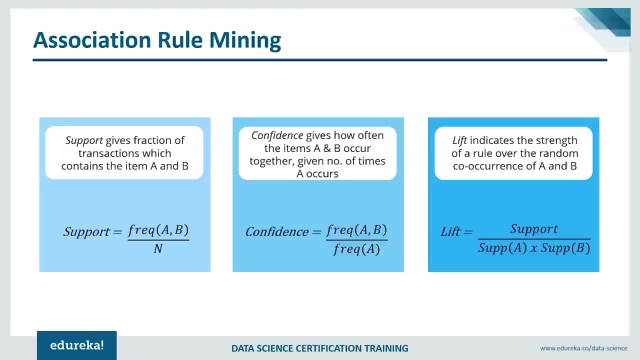 over the random co-occurrence of a and b. if you have a close look at the denominator of the lift formula, here we have support a into support b. now, a major thing which can be noted from this is that the support of a and b are independent here. so if the value of lift or the denominator 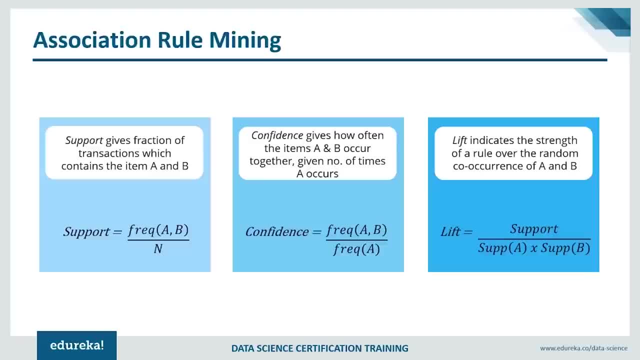 value of the lift is more, it means that the items are independently selling more, not together, so that in turn will decrease the value of lift. so what happens is that, suppose the value of lift is more, that implies that the rule which we get, it implies that the rule is strong and it can be. 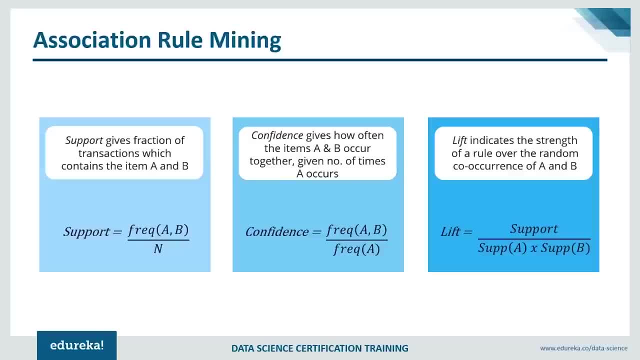 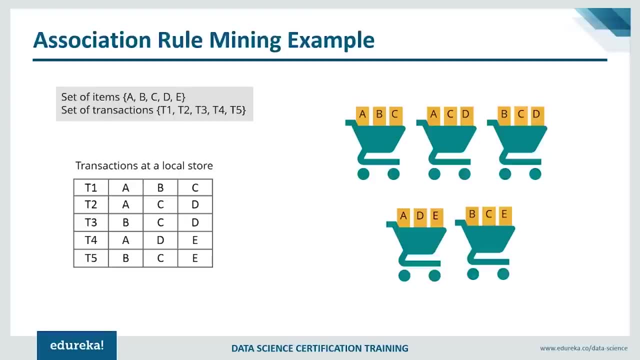 used for later purposes, because in that case the support a into support b value, which is the denominator of lift, will be low, which in turn means that there's a relationship between the items a and b. so let's take an example of association rule mining and understand how 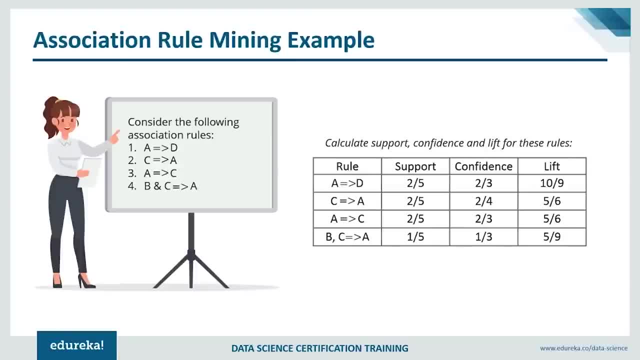 exactly it works. so let's suppose we have a set of items a, b, c, d and e and we have the set of transactions which are t1, t2, t3, t4 and t5, and what we need to do is create some sort of rules. for example, you can see: 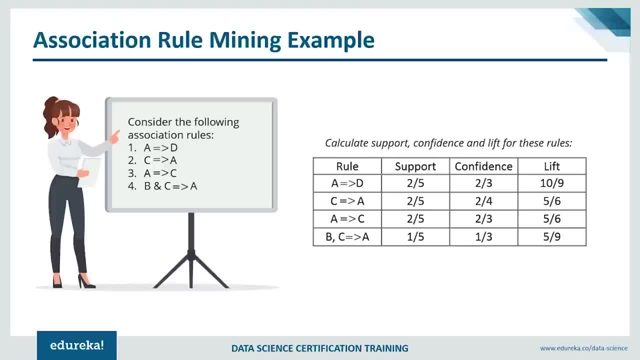 a, d, which means that if a person buys a, he buys d. if a person buys c, he buys a. if a person buys a, he buys c. and for the fourth one is: if a person by b and c, he'll in turn by a. now what we need to do? is calculate the number of items a, b, c, d and e, and we have the set of items a, b, c, d and e and we have the set of items a, b, c, d and e. and we have the set of items a, b, c, d and e and we have the support. 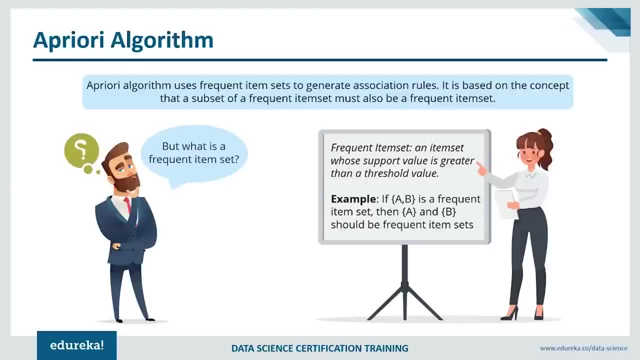 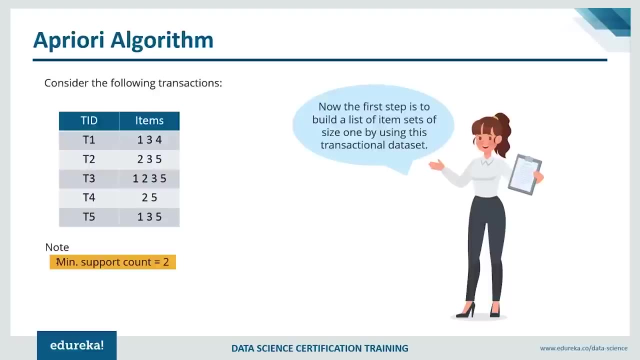 confidence and lift of these rules. now, here again, we talk about a priory algorithm. so a priory algorithm and the association rule mining go hand in hand. so what a priory does is algorithm. it uses the frequent item sets to generate the association rules and it is based 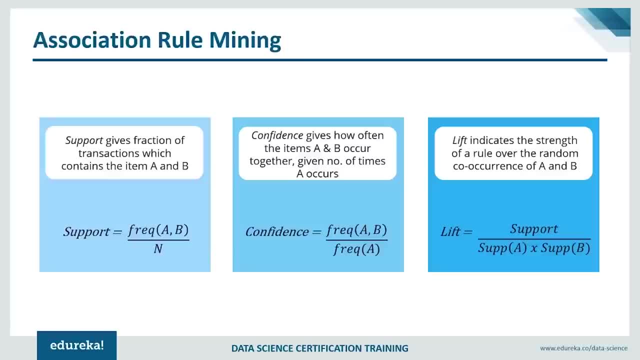 If you have a close look at the denominator of the lift formula. here we have support A into support B. Now a major thing which can be noted from this is that the support of A and B are independent here. So if the value of lift or the 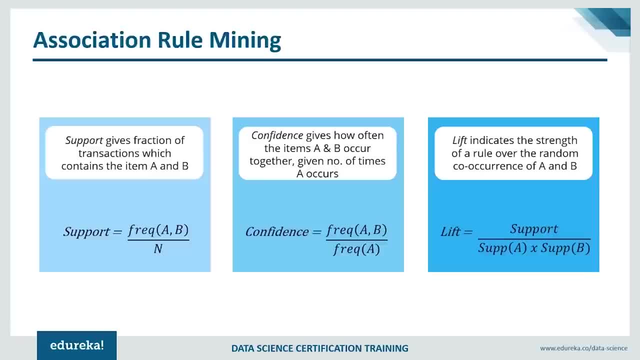 denominator value of the lift is more, it means that the items are independently selling more, not together, So that in turn will decrease the value of lift. So what happens is that, suppose the value of lift is more, that implies that the rule which we get, it implies that the rule is strong and it can. 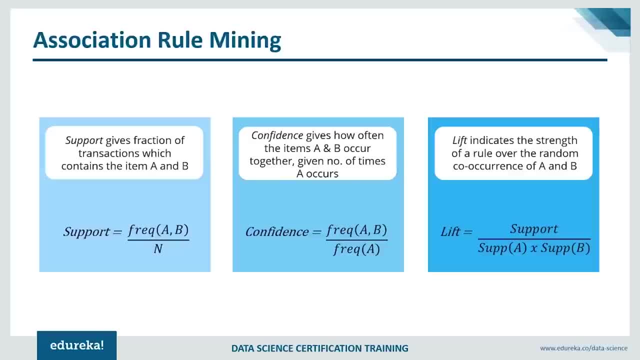 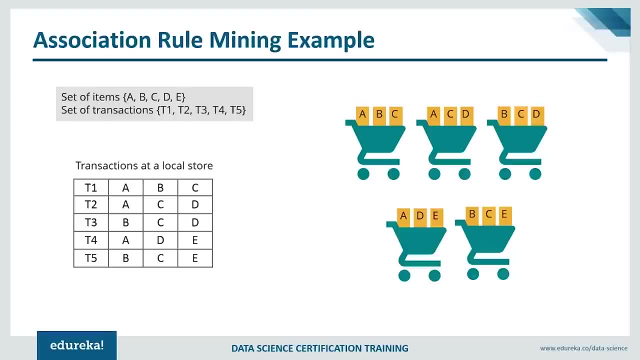 be used for later purposes, because in that case the support A into support B value, which is the denominator of lift, will be low, which in turn means that there's a relationship between the items A and B. So let's take an example of association rule mining and understand how. 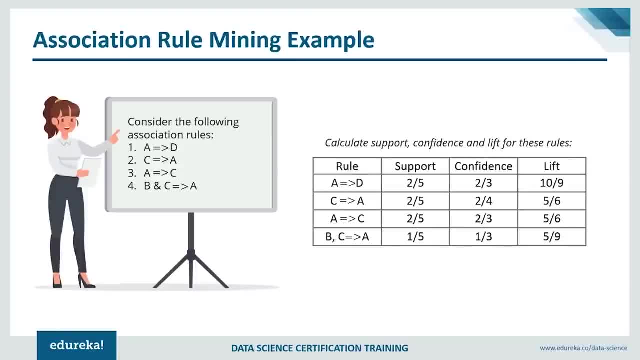 exactly it works. So let's suppose we have a set of items A, B, C, D and E and we have the set of transactions which are T1, T2, T3, T4 and T5 and what we need to. 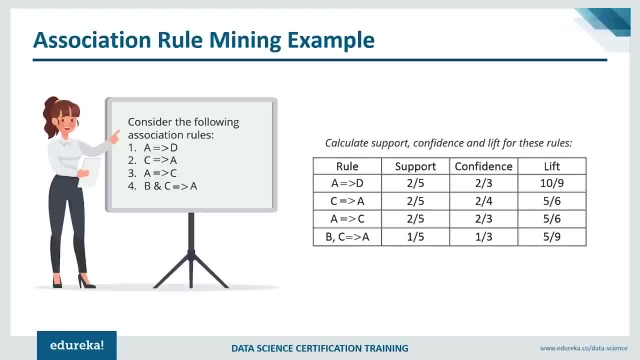 do is create some sort of rules. For example, you can see A- D, which means that if a person buys A, he buys D. If a person buys C, he buys A. If a person buys A, he buys A. And for the fourth one is: if a person buys B and C, he'll in turn buy A. 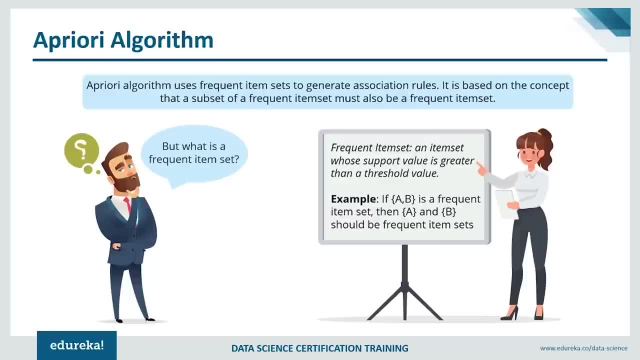 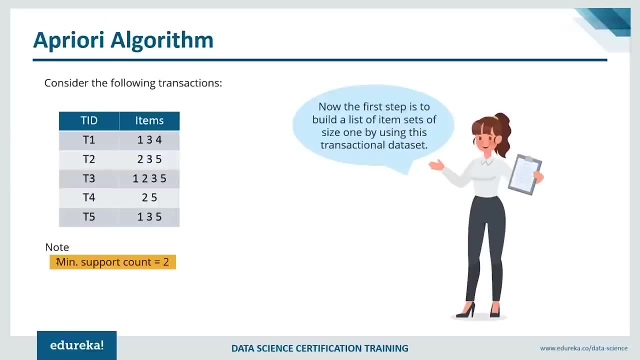 Now what we need to do is calculate the support, confidence and lift of these rules. Now, here again we talk about a priori algorithm. So a priori algorithm and the association rule mining go hand in hand. So what a priori does is algorithm. it uses the frequent item sets to 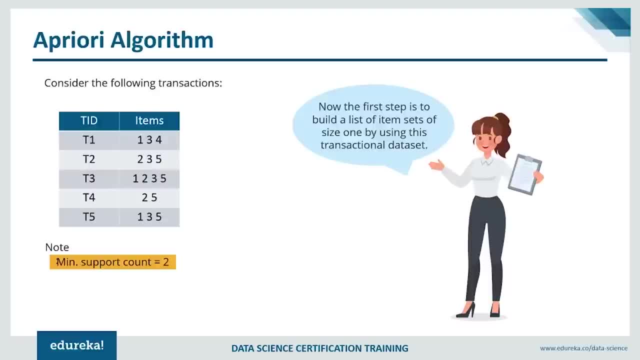 generate the association rules and it is based on the concept that a subset of a frequent item set must also be a frequent item set. So let's understand what is a frequent item set and how all of these work together. So if we take the following transactions of items, we have transaction T1 to 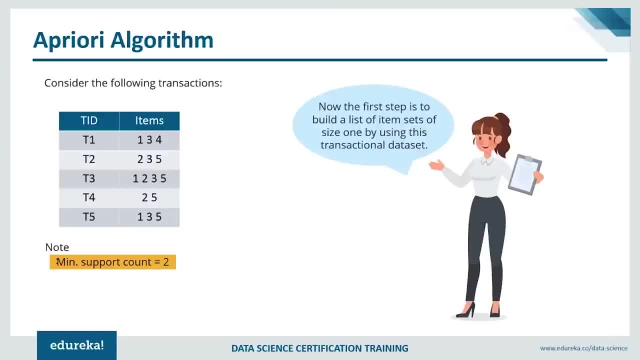 T5 and the items are 1, 3, 4,, 2, 3, 5,, 1, 2, 3, 5, 2, 5 and 1, 3, 5.. 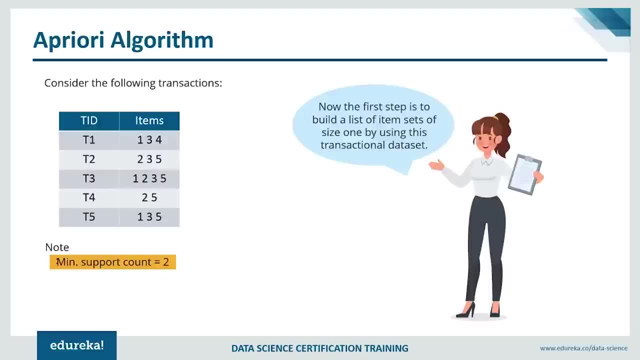 on the concept that a subset of a frequent item set must also be a frequent isom set. so let's understand what is a frequent item set and how all of these work together. if we take the following transactions of items, we have transaction t1 to t5 and the items are: 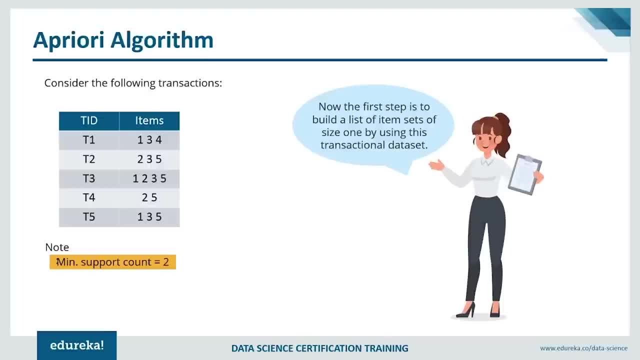 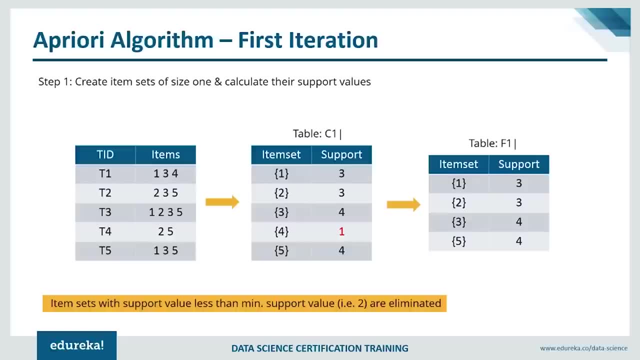 1, 3, 4, 2, 3, 5, 1, 2, 3, 5, 2, 5 and 1 3, 5. now, another more important thing about support which i forgot to mention was that when talking about association rule mining, there is a minimum. 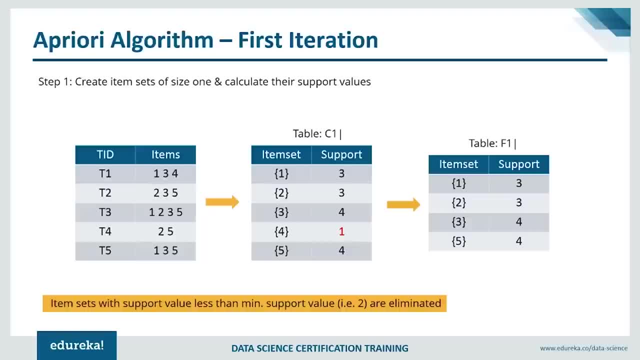 support count. what we need to do now, the first step, is to build a list of item set of size one using this transaction data set and use the minimum support count 2. now let's see how we do that. if we create the table c1, if you have a close look at the table c1, we have the item set. 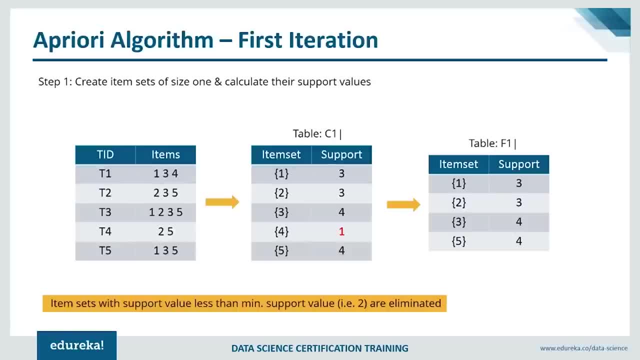 1, which has a support, 3, because it appears in the transaction- 1, 3 and 5. similarly, if we have a look at the item set, the single item, 3, so it has a support of 4. it appears in t1, t2, t3 and t5. but 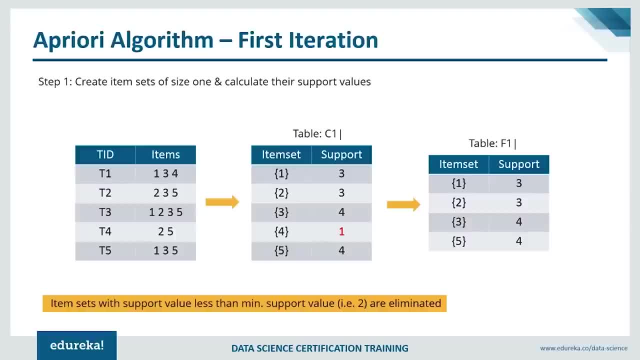 if we have a look at the item set 4, you can see that the item set 1 has a support of 3 and the item set 2 has a support of 4. it only appears in the transaction one, so its support value is one. now, the item set with the 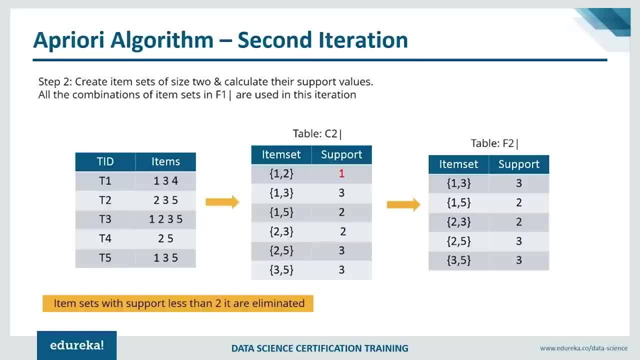 support value which is less than the minimum support value, that is, 2, have to be eliminated. so the final table, which is a table f1, has one, two, three and five. it does not contain the four. now what we're going to do is create the item list of the size two and all the combination of 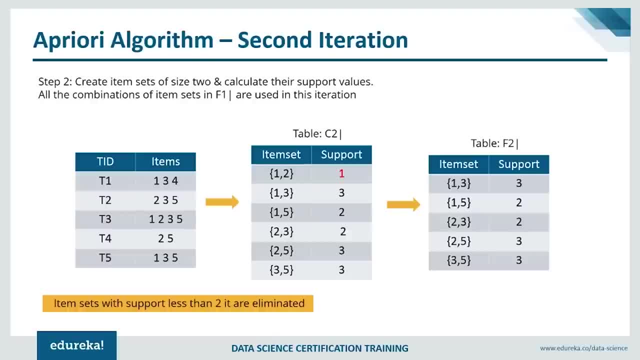 the item sets in f1 are used in this iteration, so we've left four behind. we just have one, two, three and five. so the possible item sets are one, two, one three, one five, two, three, two, five and three, five. then again we'll calculate the support. so in this case, if we have a closer look at the table c2, 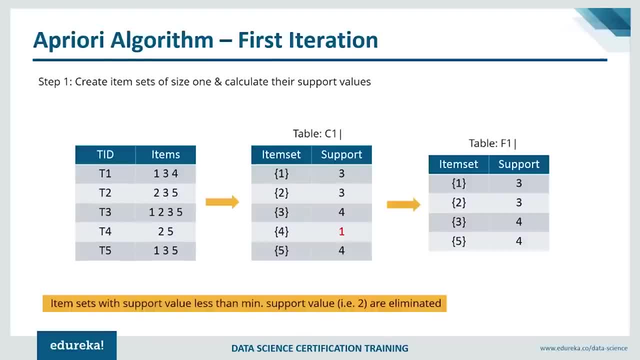 Now, another more important thing about support, which I forgot to mention, was that when talking about association rule, mining Is a minimum support count. what we need to do Now, the first step, is to build a list of item set of size 1 using this: 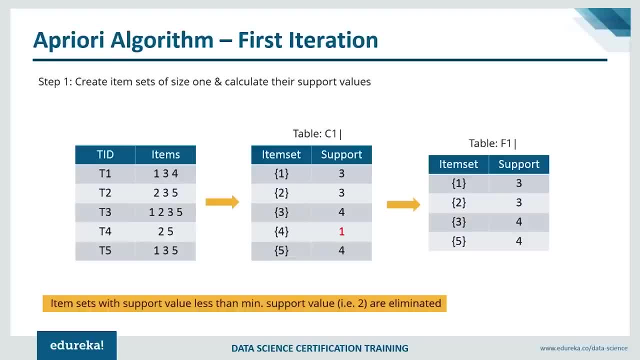 transaction data set and use the minimum support, count 2.. Now let's see how we do that. If we create the table C1, if you have a close look at the table C1, we have the item set 1, which has a support 3 because it appears in the 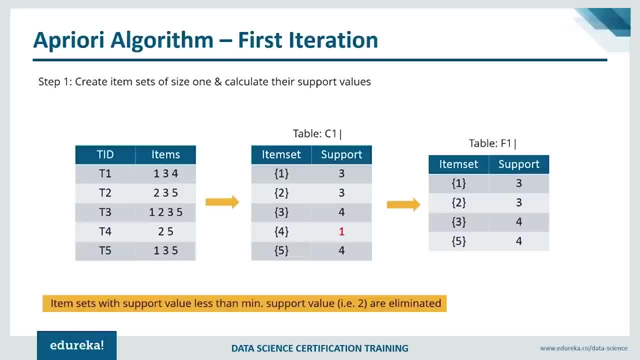 transaction 1, 3 and 5.. Similarly, if you have a look at the item set, the single item 3, so it has a support of 4. It appears in T1,, T2,, T3 and T5.. 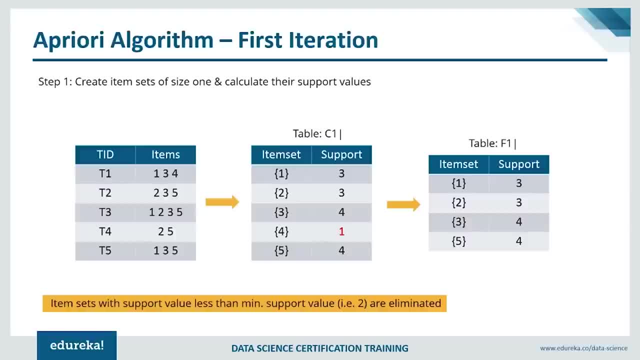 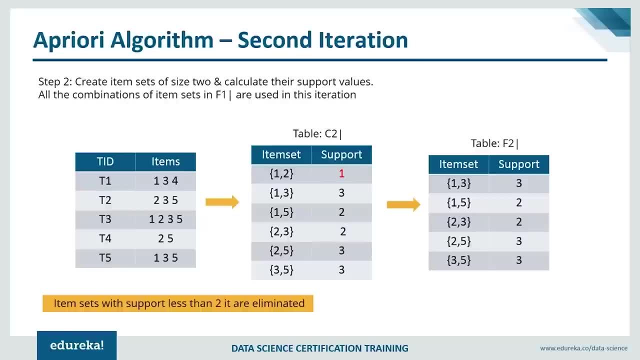 But if we have a look at the item set 4, it only appears in the transaction 1.. So its support value is 1.. Now the item set with the support value which is less than the minimum support value, that is, 2, have to be eliminated. 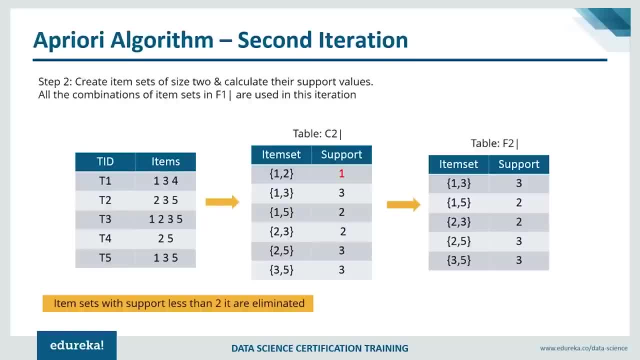 So the final table, which is a table F1, has 1,, 2,, 3 and 5.. It does not contain the 4.. Now what we're going to do is create the item list of the size 2 and all. 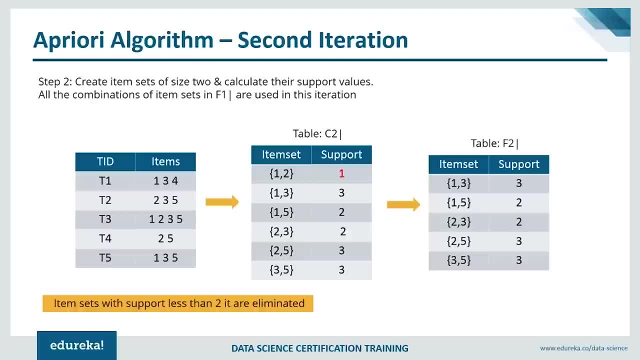 the combination of the Item sets in F1 are used in this iteration, So we've left 4 behind. We just have 1, 2, 3 and 5.. So the possible item sets are 1, 2, 1, 3, 1, 5, 2, 3, 2, 5 and 3, 5.. 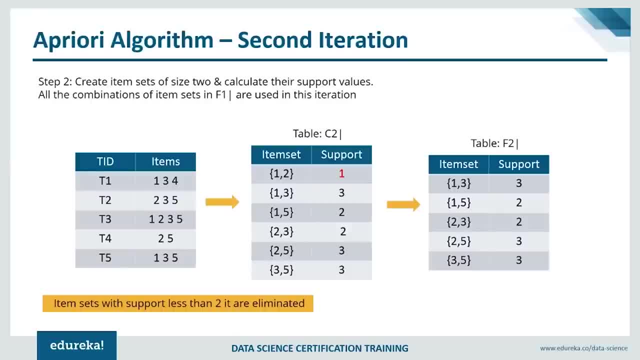 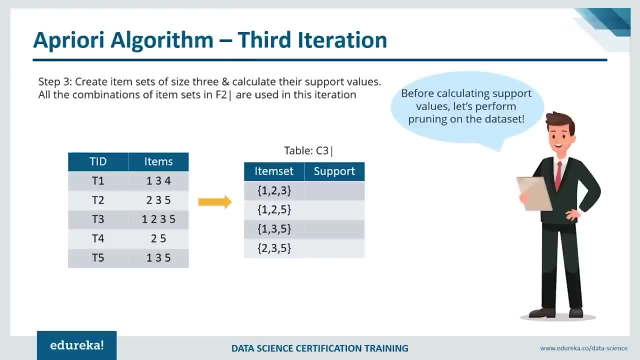 Then again we'll calculate the support. So in this case, if you have a closer look at the table C2, we see that the item set 1, 2 is having a support value 1, which has to be eliminated. So the final table F2 does not contain 1, 2.. 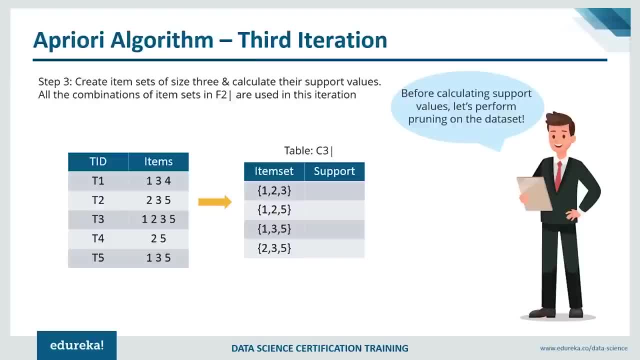 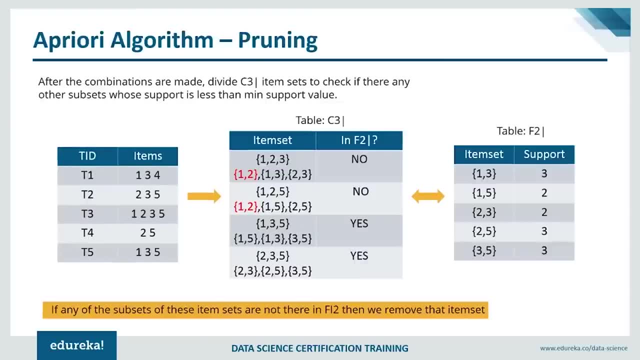 we see that the item set one comma two is having a support value, one which has to be eliminated. so the final table f2 does not contain one comma two. similarly, if we create the item sets of size three and calculate the support values, but before calculating the support, let's perform the peering on the data set. now, what's peering? so? 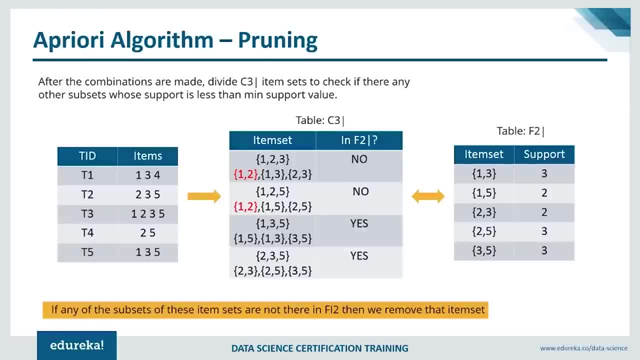 after all the combinations are made, we divide the table c3 items to check if there are another subset whose support is less than the minimum support value. this is a priori algorithm. so in the item sets one, two, three, what we can see? that we have one, two and in the one, two, five. 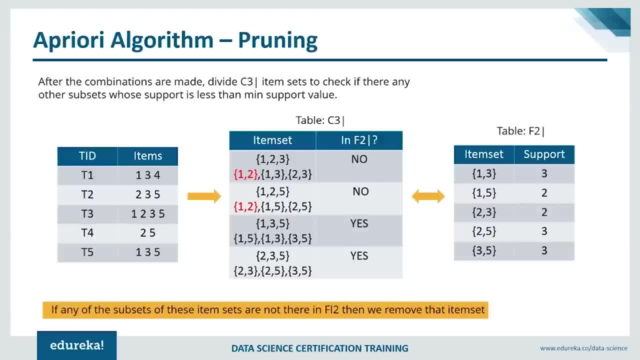 again we have one, two. so we'll discard both of these item sets and we'll be left with the same, with one, three, five and two, three, five. so with one, three, five, we have three subsets- one, five, one, three, three, five, which are present in table f2. then again we have two, three, two, five and three. 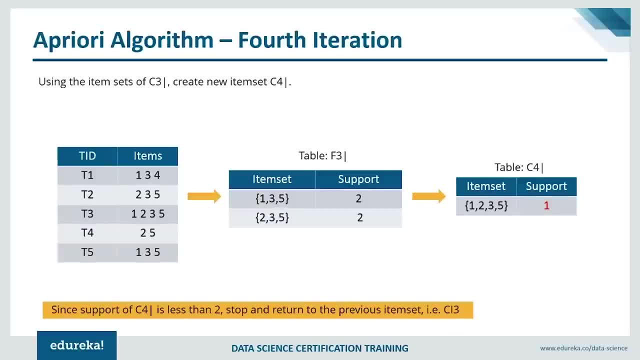 five, which are also present in table f2. so we have to remove one comma two from the table c3 and create the table f3 now if we're using the items of c3 to create the items of c4. so what we find is that we have the item set one. 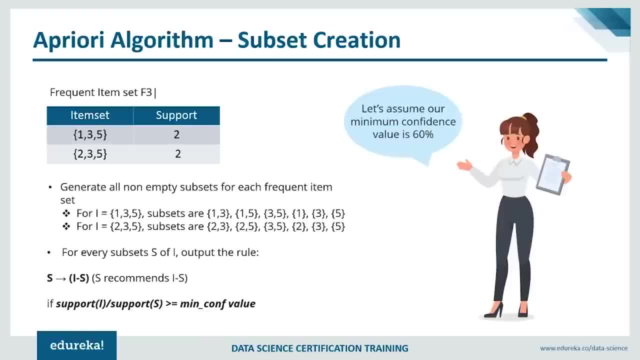 two, three, five. the support value is one which is less than the minimum support value of two. so what we're going to do is stop here and we're going to return to the previous item set, that is, the table c3. so the final table f3 was 1, 3, 5 with the support value of 2 and 2, 3, 5 with a support. 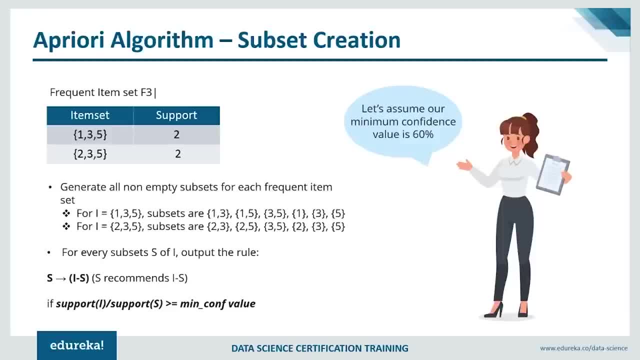 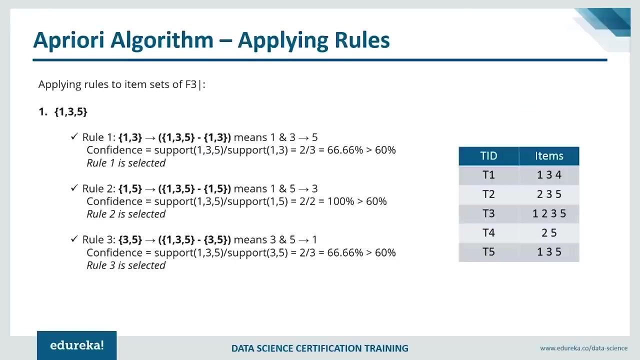 value of 2.. now what we're going to do is generate all the subsets of each frequent item sets. so let's assume that our minimum confidence value is 60 percent. so for every subset s of i, the output rule is: that s gives i to s. is that s recommends i n s. if the support of i divided by the support of s is greater than. 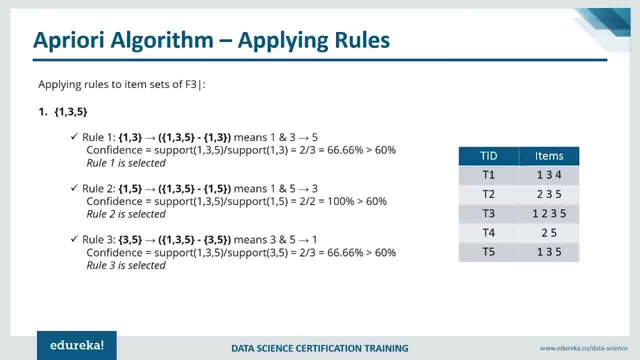 or equal to the minimum confidence value, then only will proceed further. so keep in mind that we have not used lift till now. we are only working with support and confidence. so applying rules with item sets of f3 we get rule one, which is one comma three, which gives one three, five and one three. 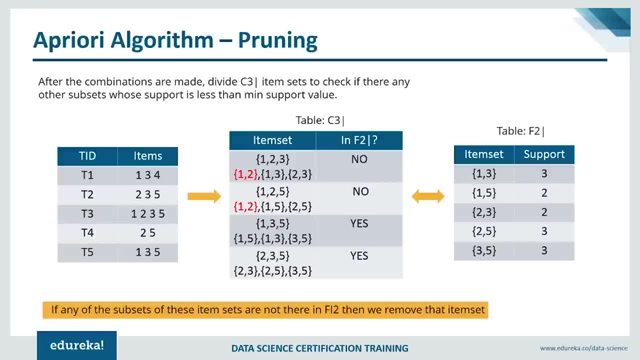 Similarly, if we create the item sets of size 3 and calculate the support values. but before calculating the support, let's perform the peering on the data set. Now, what's peering? So, after all the combinations are made, we divide the table C3 items to: 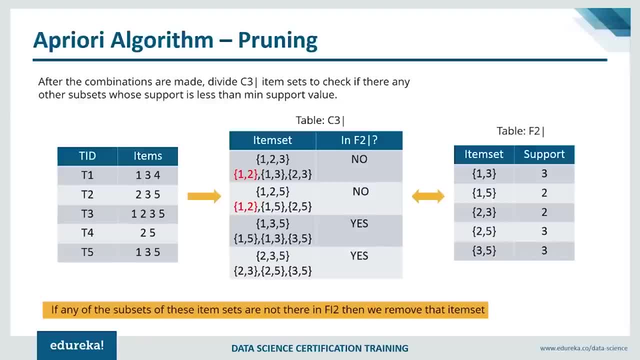 check if there are another subset whose support is less than the minimum support value. This is a priori algorithm. So in the item sets 1,, 2,, 3, what we can see, that we have 1,, 2, and in the 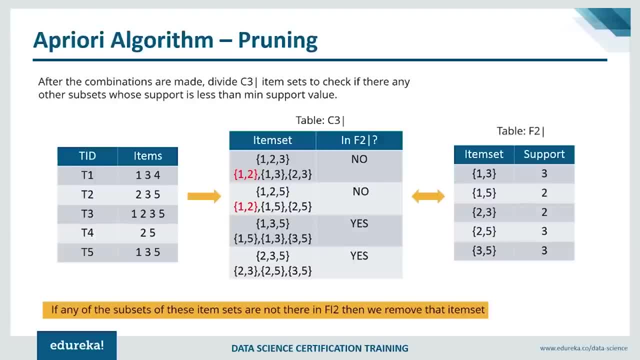 1, 2, 5.. Again, we have 1, 2.. So we'll discard both of these item sets and we'll be left with 1, 3, 5 and 2, 3, 5.. 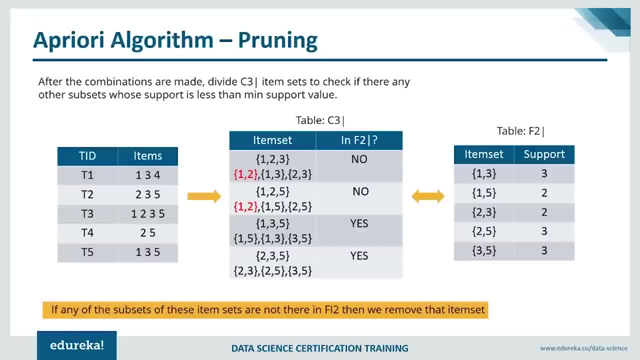 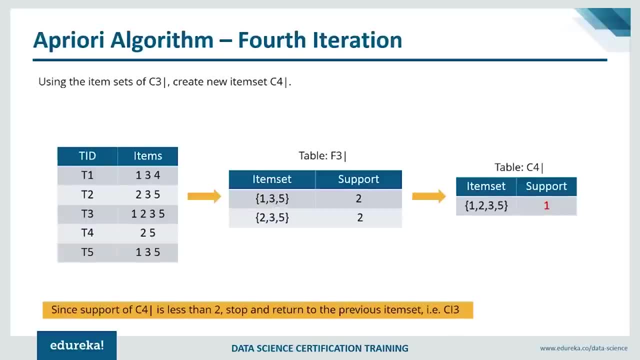 So with 1, 3, 5, we have three subsets: 1, 5,, 1, 3, 3, 5, which are present in table F2.. Then again we have 2, 3,, 2, 5 and 3, 5, which are also present in table F2.. 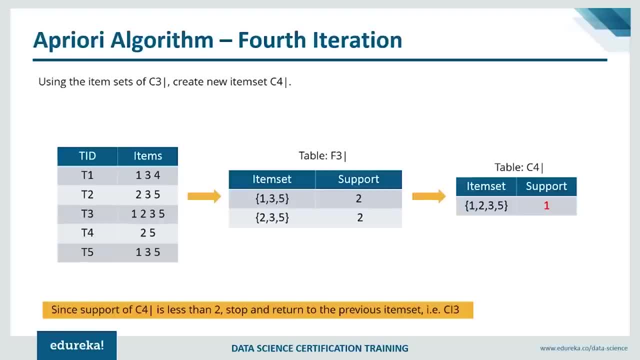 So we have to remove 1, 2 from the table C3 and create the table F3.. Now, if you're using the items Of C3 to create the items of C4. So what we find is that we have the item set 1, 2, 3, 5.. 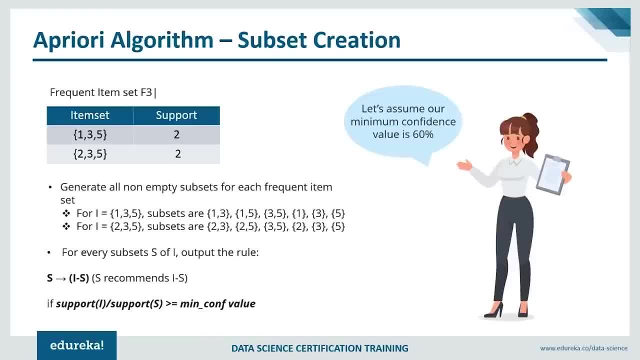 The support value is 1, which is less than the minimum support value of 2.. So what we're going to do is stop here and we're going to return to the previous item set, That is, the table C3.. So the final table F3 was 1, 3, 5 with the support value of 2 and 2, 3, 5. 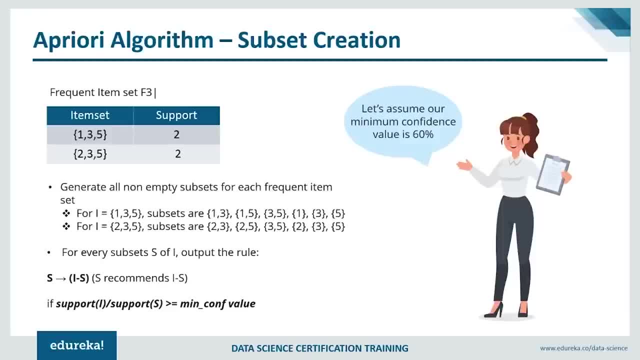 with a support value of 2.. Now what we're going to do is generate all the subsets Of each frequent item sets. So let's assume that our minimum confidence value is 60%. So for every subset S of I, the output rule is that S gives I to S. is that S. 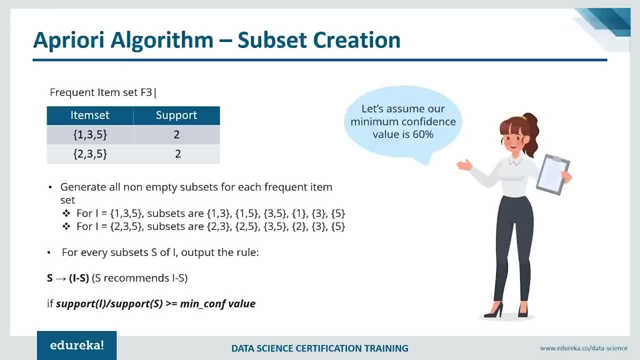 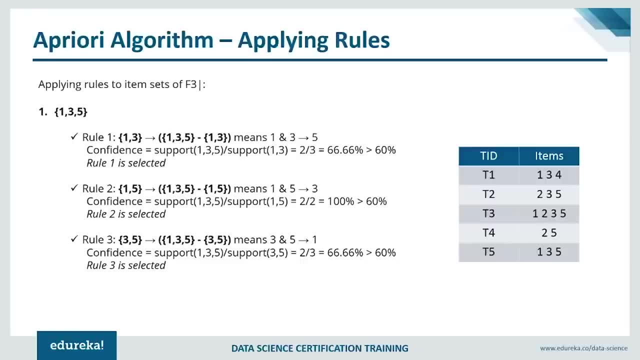 recommends I and S. If the support of I divided by the support of S is greater than or equal to the minimum confidence value, then only will proceed further. So keep in mind that we have not used lift till now, We are only working. 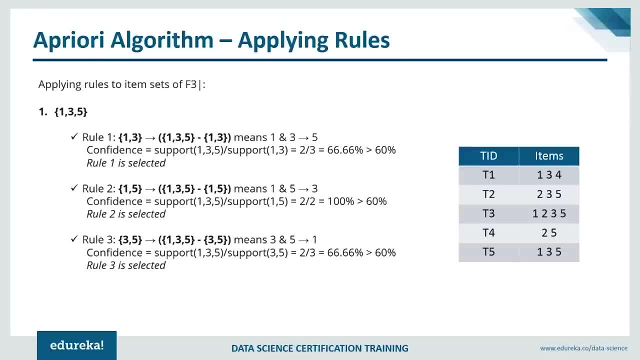 With support and confidence. So, applying rules to the item sets of F3, we get rule 1,, which is 1, 3, which gives 1, 3, 5 and 1, 3.. It means if you buy 1 and 3, there's a 66% chance that you'll buy item 5 also. 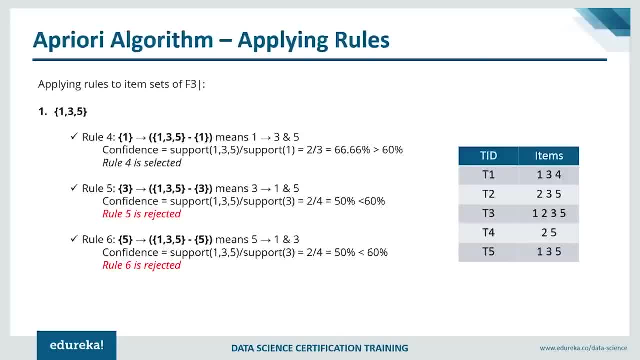 Similarly, the rule 1, 5.. It means that if you buy 1 and 5, there's 100% chance that you will buy 3 also. Similarly, if we have a look at rule 5. And 6, here the confidence value is less than 60%, which was the assumed. 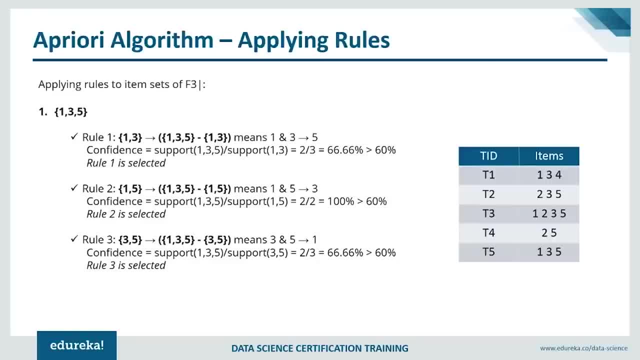 it means if you buy one and three, there's a 66 percent chance that you'll buy item five also. similarly, the rule one comma five. it means that if you buy one and five, there's hundred percent chance that you will buy three also. similarly, if we have a look at rule five and six here, the 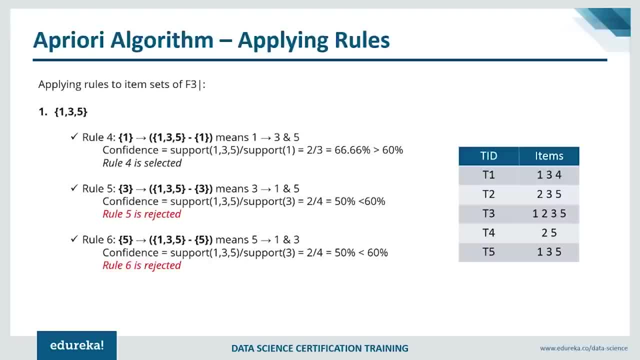 confidence value is less than sixty percent, which was the assumed confidence value. so what we're going to do is we'll reject these files now. an important thing to note here is that have a closer look to the rule five and rule three. you see it has one five, three. 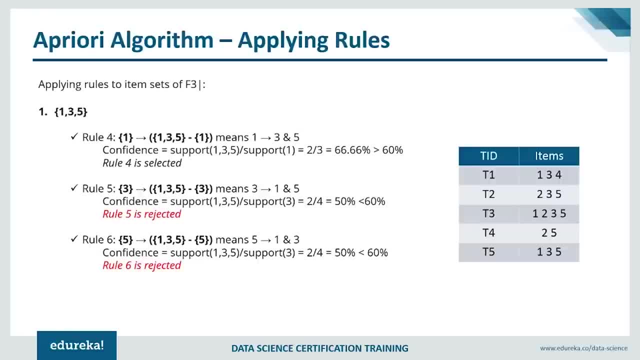 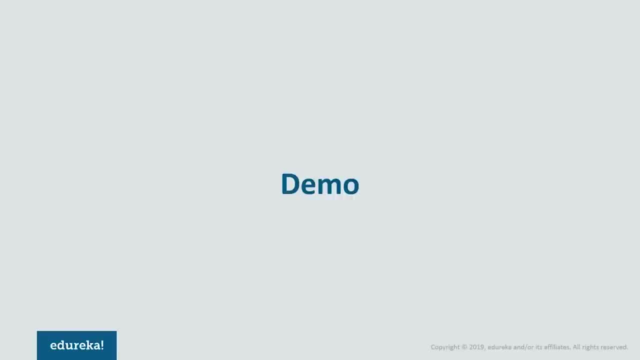 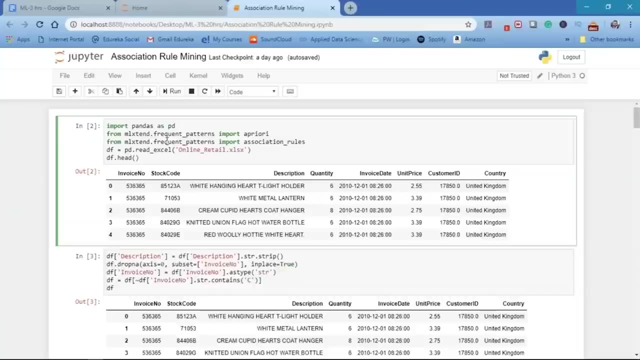 one five, three, three, one, five. it's very confusing. so one thing to keep in mind is that the order of the item sets is also very important. that will help us allow, create good rules and avoid any kind of confusion. so that's that. so now let's learn how association rule view is important. 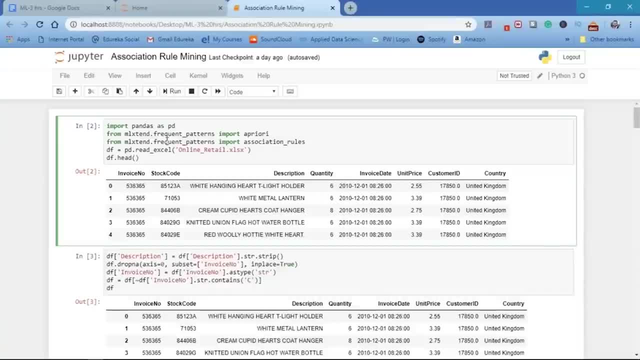 used in market basket analysis problems. so what we'll do is we'll be using the online transactional data of a retail store for generating association rules. so, first of all, what you need to do is import pandas, MLT, ML, XT and E libraries from the imported and read the data. so, first of all, what we're gonna do is read: 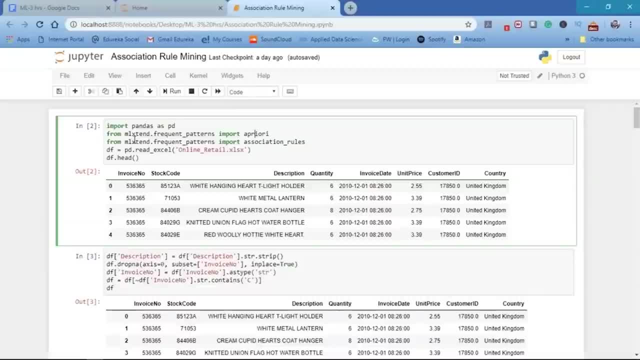 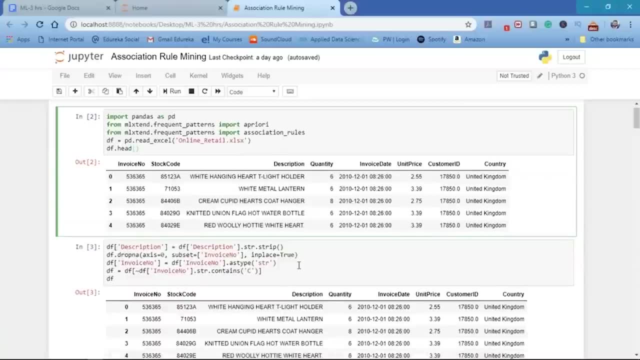 the data. what we're gonna do is, from ML, XT and E dot frequent patterns, we're going to improve the a priority and the association rules. as you can see, here we have the head of the data. you see, we have inverse number, stock code, the description, quantity, the inverse detail, unit, price, custom ID and the country. so 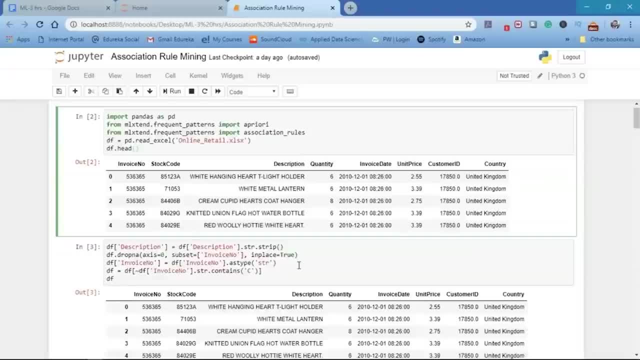 in the next step. what we will do is we will do the data cleanup, which includes living spaces from some of the descriptions given, and what we're going to do is drop the rules that do not have the inverse numbers and remove the credit transaction. so, hey, what? what you're gonna do is 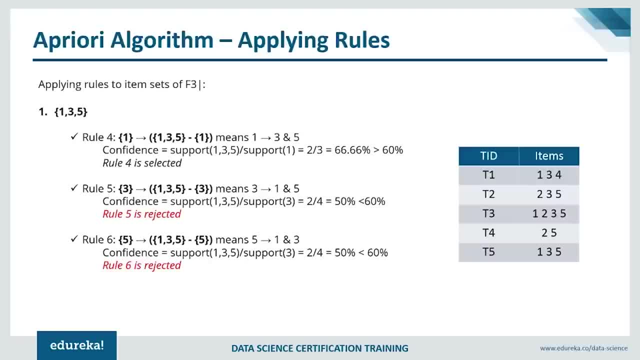 confidence value. So what we're going to do is we'll reject these files. Now, an important thing to note here is that have a closer look to the rule 5 and rule 3.. You see it has 1, 5, 3, 1, 5, 3, 3, 1, 5.. 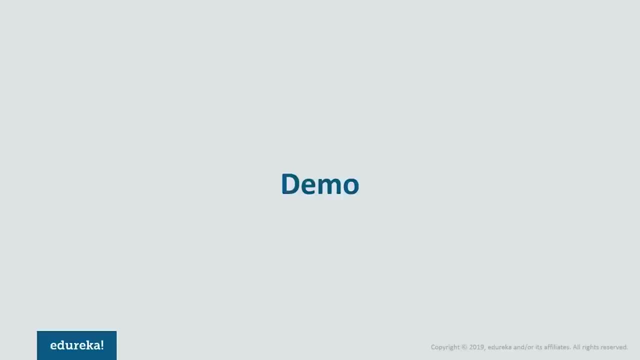 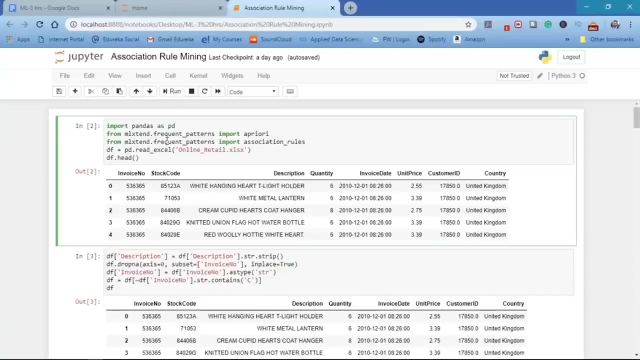 It's very confusing. So one thing to keep in mind is that the order of the item sets is also very important. that will help us allow create good rules. So that's that. So now let's learn how association rule are used in market basket analysis problems. 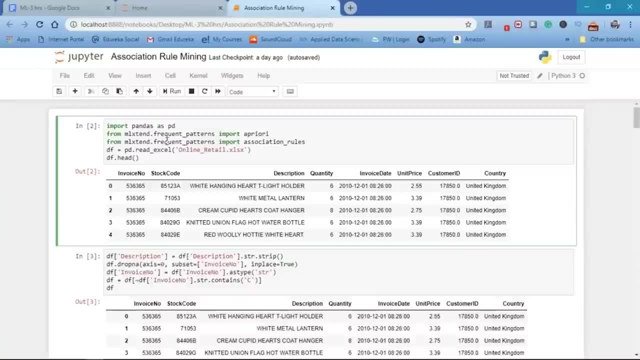 So what we'll do is we'll be using the online transactional data of a retail store for generating association rules. So, first of all, what you need to do is import Pandas, MLT, MLX, D&D libraries from the imported and read the data. 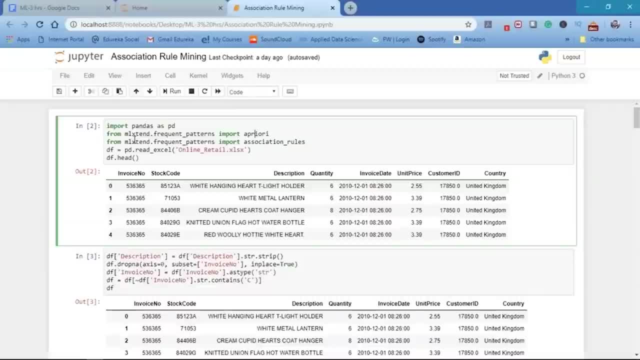 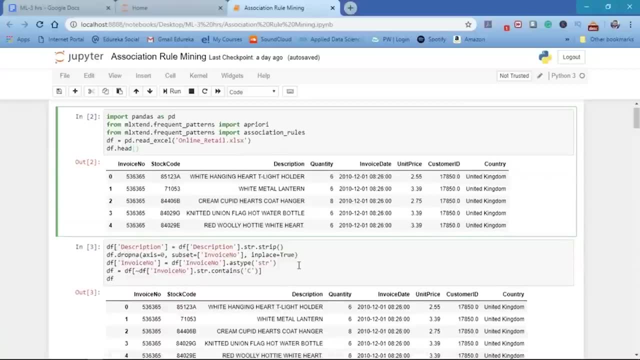 So, first of all, what we're going to do is read the data. What we're going to do is, From MLX, D&D, dot, frequent patterns, We're going to improve the a priori and the association rules. As you can see, here we have the head of the data. 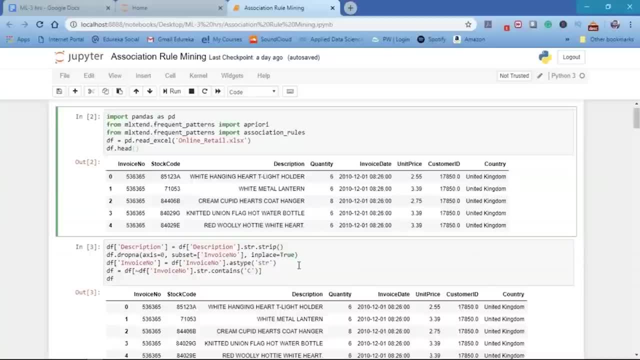 You see, we have inverse numbers, stock code, the description, quantity, the inverse detail, unit, price, customer ID and the country. So in the next step, what we will do is we will do the data cleanup, which includes removing spaces from some of the descriptions given, and what we're 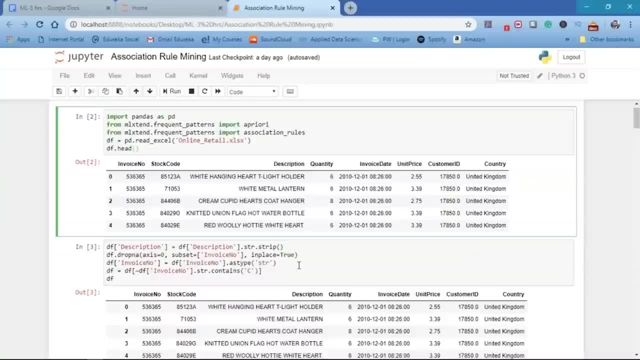 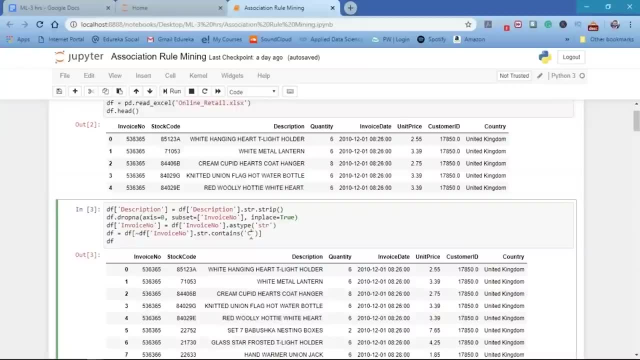 going to do is drop the rules that do not have the inverse numbers and remove the credit. So here, what we're going to do is remove which do not have an inverse number. If the string contains type- scene was a number, then we're going to remove that. 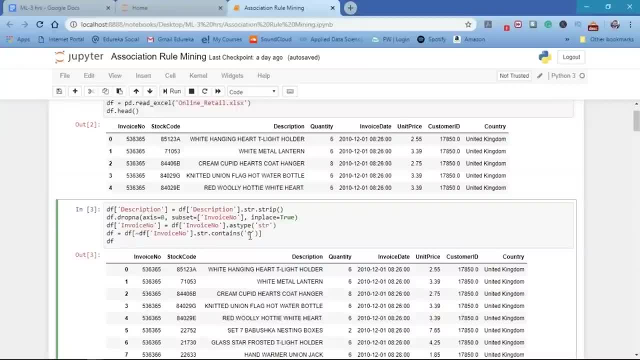 remove the credit transactions and remove the registration data from the the credit transactions. so, hey, what? what you're gonna do is remove the remove which do not have an inverse number. if the string contains type seen was a number, then we're going to remove that. those are the credits. remove any. 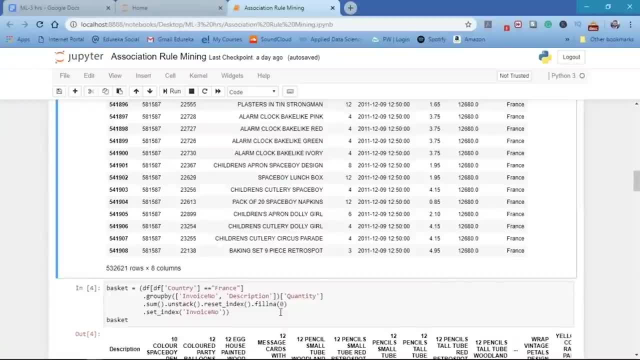 Those are the credits. remove any kind of spaces from the descriptions. So, as you can see, here we have like 532,000 rows with eight columns. So next, what we're going to do is, after the cleanup, we need to consolidate the items. 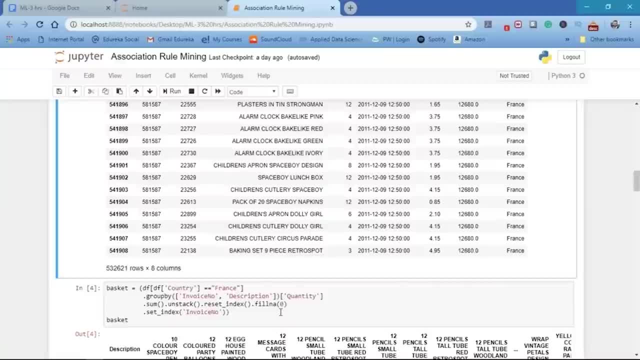 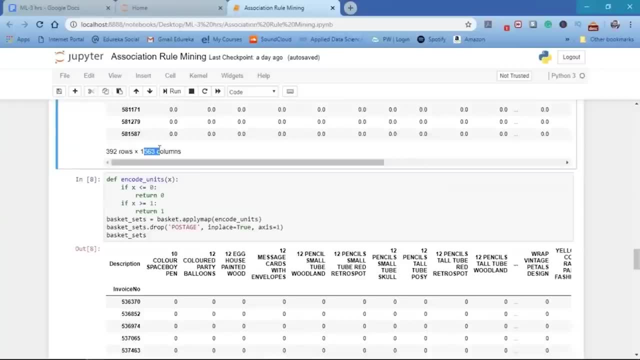 into one transaction per row with each product for the sake, And so we're going to do that. So now, if we want to keep the data set small, we want to only look at the saves for France, So we're going to use the only France and group by invoice number description. 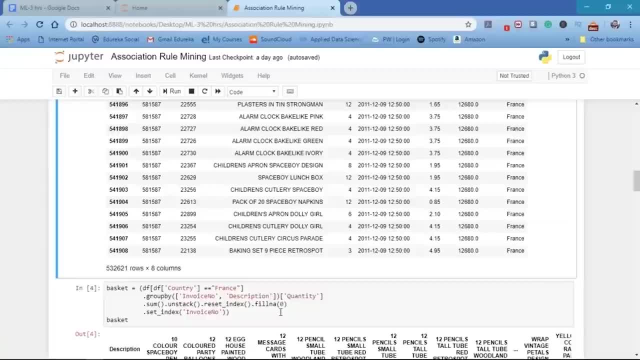 kind of spaces from the descriptions. so, as you can see, here we have like 532 thousand rows with eight columns. so next, what we're going to do is, after the cleanup, we need to consolidate the items into one transaction per row with each product. for the sake of keeping the data set small. we want to only look at the 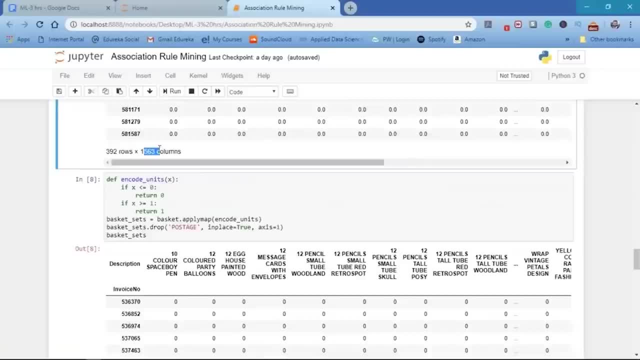 sales for France. so we're going to use the only France and group by invoice number description with the quantity. sum up and see so, which leaves us with 392 rows and 1563 columns. now there are a lot of zeros in the data, but we also 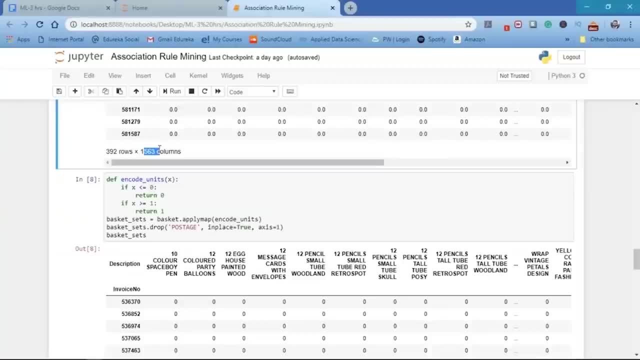 need to make sure any positive values are converted to a 1 and anything less than 0 is set to 0. so for that we're going to use this code defining encode units. if X is less than 0, it on 0 if X is greater. 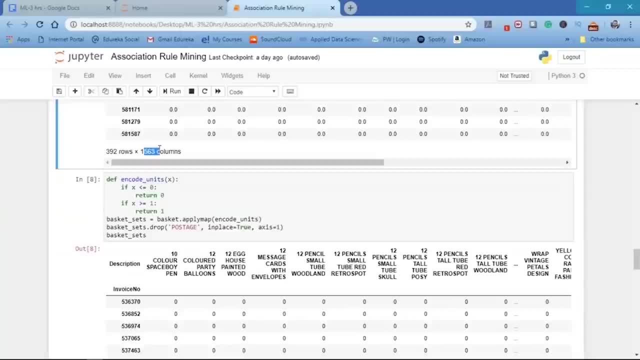 than 1, return 1. so what we're going to do is map and apply it to the whole data set we have here. so, now that we have structured the data properly, so the next step is to generate the frequent item set that has support of at least 7%. now, 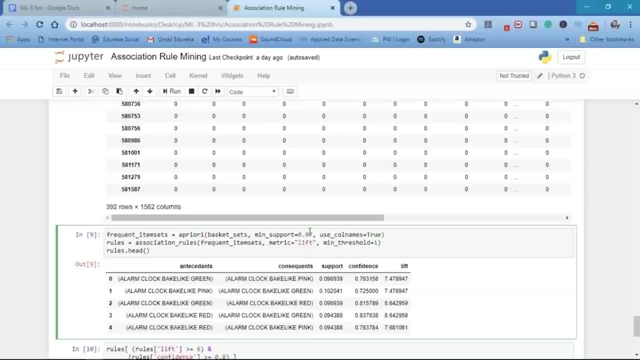 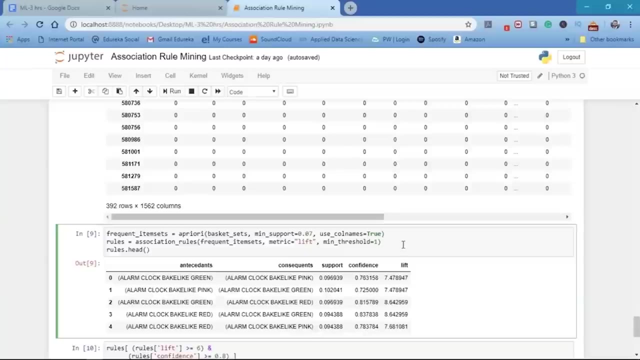 this number is chosen so that you can get close enough. now what we're going to do is generate the rules with the corresponding support, confidence and lift. so we have given the minimum support as 0.7. the metric is left free when I'll set, and threshold is 1. so these are the following rules. now a few. 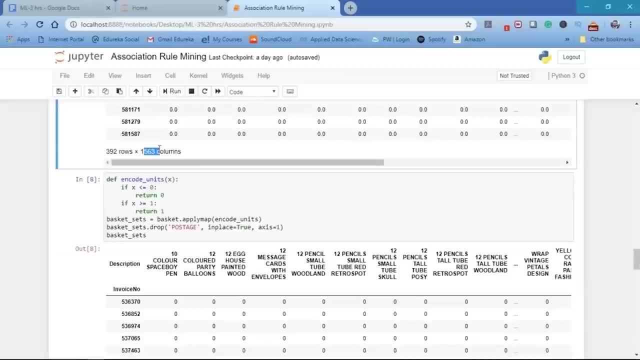 with the quantity, sum up and see So, which leaves us with 392 rows and 1563 columns. Now there are a lot of zeros in the data, but we also need to make sure any positive values are converted to a one and anything less than zero is set to zero. 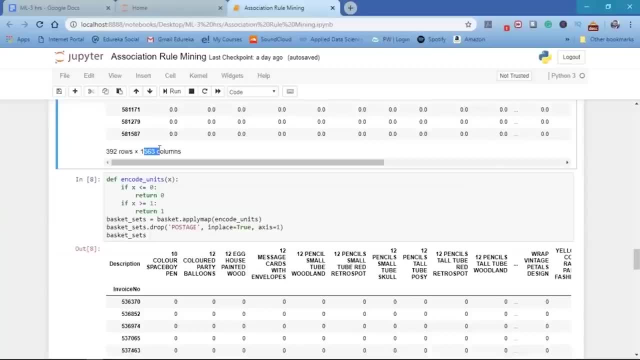 So for that we're going to use this code. So we're going to say: x is less than zero, It's all. zero effects is greater than one, return one. So what we're going to do is map and apply it to the whole data set we have here. 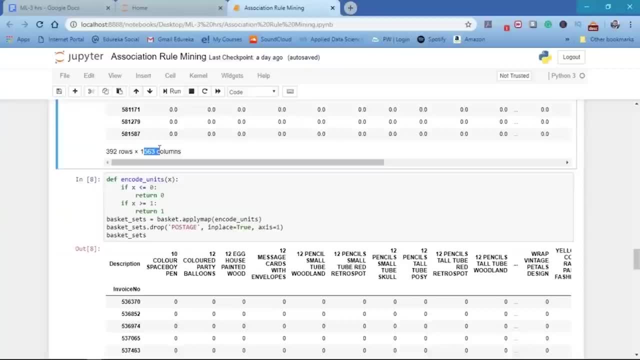 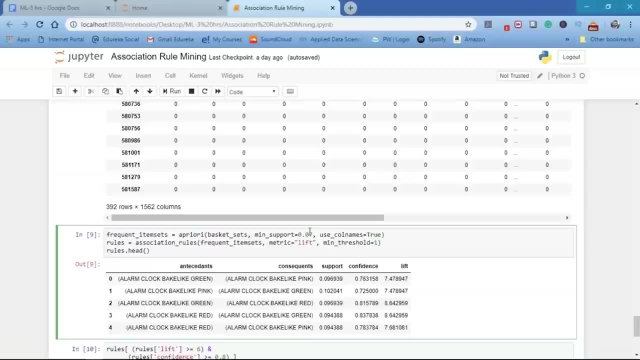 So, now that we have structure the data properly, So the next step is to generate the frequent item set that has support of at least 7%. Now, this number is chosen so that you can get close enough. Now what we're going to do is generate the rules with the corresponding support. 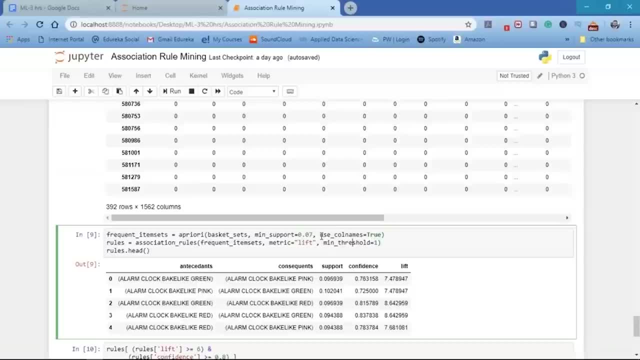 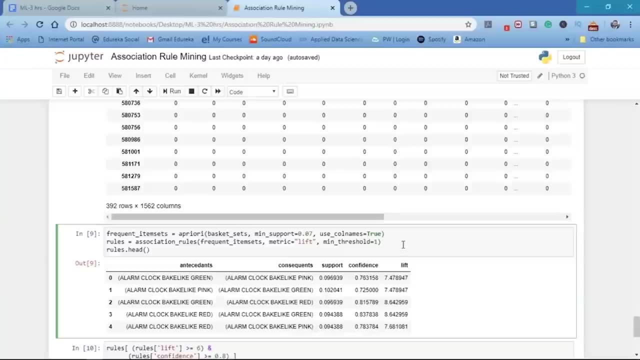 confidence and lift. So we have given The minimum support as 0.7.. The metric is left, frequent item set and threshold is one. So these are the following rules. Now a few rules with a high lift value, which means that it occurs more. 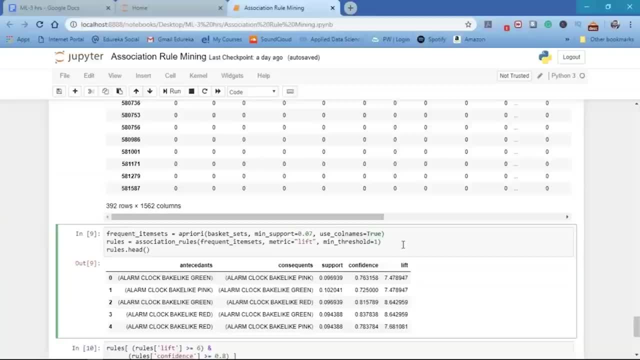 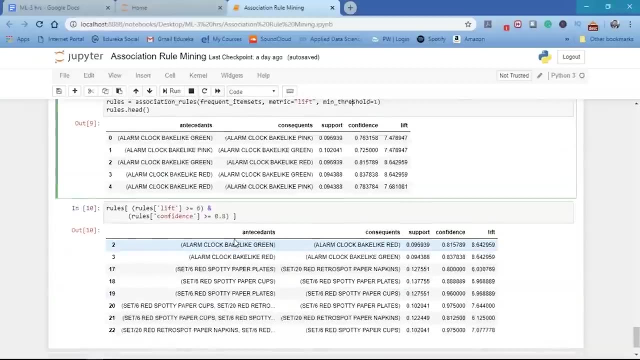 rules with a high lift value, which means that it occurs more frequently than would be expected given the number of transaction, the product combinations, most of the places, the confidence is high as well. so these are few of the observations, what we get here if we filter the data frame using the standard. 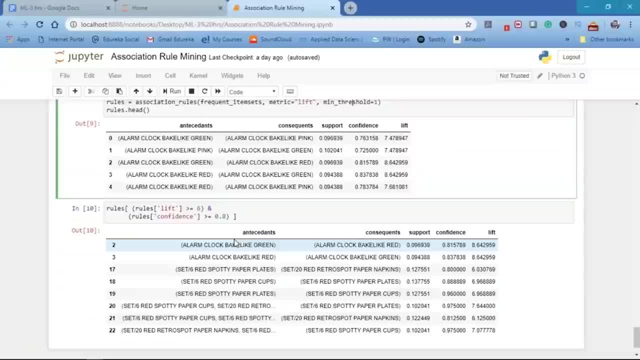 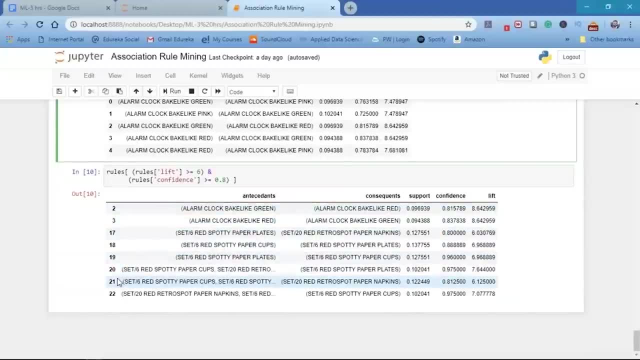 pandas code for large lift: 6 and high confidence: 0.8. this is what the output is going to look like. these are 1, 2, 3, 4, 5, 6, 7, 8. so, as you can see, here we have the age rules, which are the final rules which are given by: 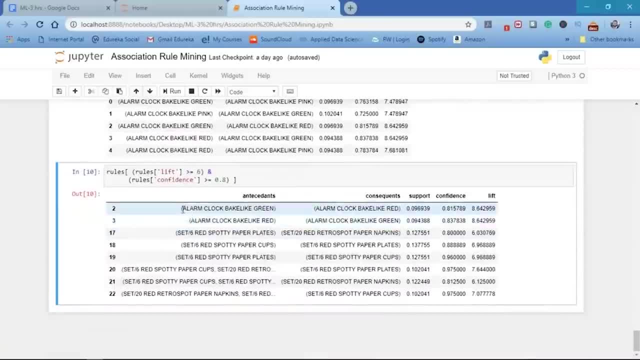 the association rule mining, and that is how all the industries, or any of these which talk about large retailers. they tend to know how their products are used and how exactly they should rearrange and provide the offers on the products so that people spend more and more time on the products and they can get more and more. 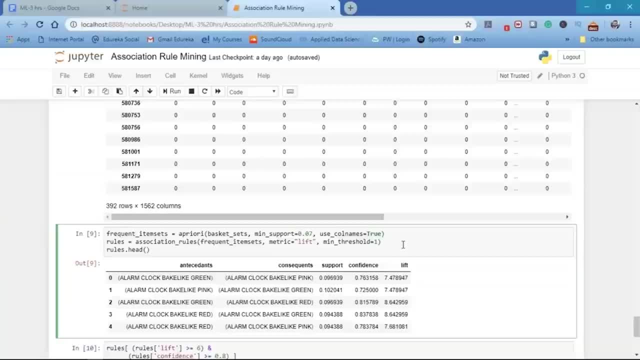 frequently than would be expected given the number of transaction, the product combinations, most of the places, the confidence is high as well. So these are few of the observations. what we get here If we filter the data frame using the standard pandas code for large lift. 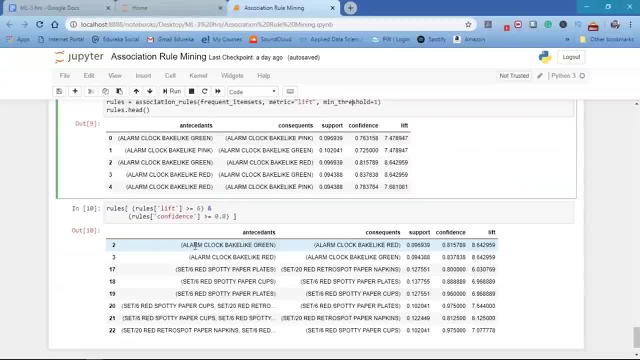 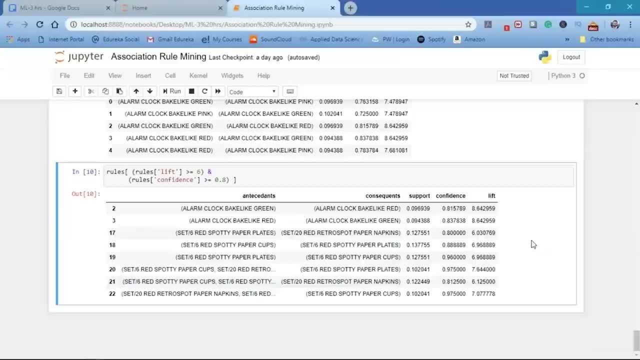 6 and high confidence, 0.8.. This is what the output is going to look like. These are 1, 2, 3, 4, 5, 6, 7, 8.. So, as you can see, here we have the age rules, which are the final rules which are given. 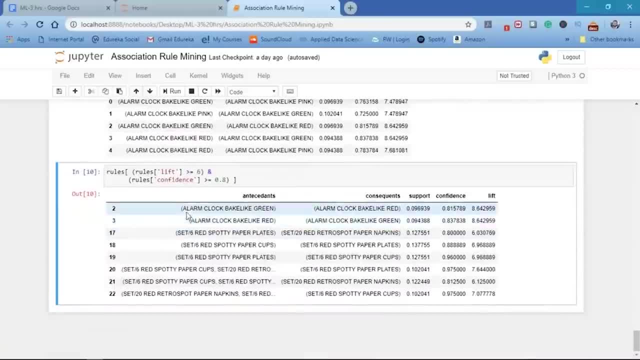 by the association rule mining, and that is how all the industries or any of these which talk about large retailers. They tend to know how their products are used and how exactly they should rearrange and provide The offers on the product so that people spend more and more money and time in the shop. 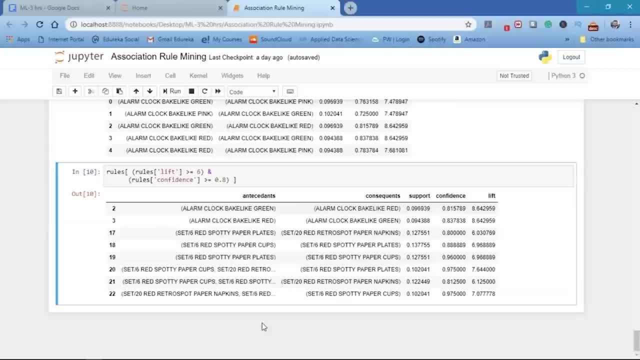 So that was all about association rule mining. So so, guys, that's all for unsupervised learning. I hope you got to know about the different formulas, how unsupervised learning works, because you know we did not provide any label to the data. 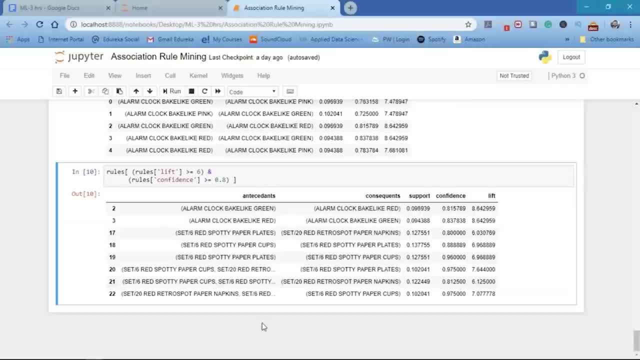 money and time in the shop. so that was all about association rule mining. so so, guys, that's all for unsupervised learning. I hope you got to know about the different formulas, how unsupervised learning works, because you know we did not provide any label to the data. all we did was create some rules and not 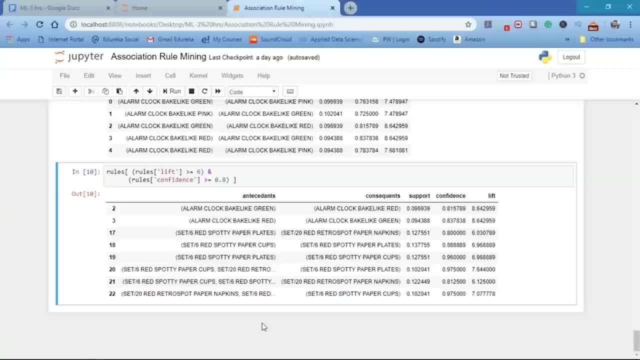 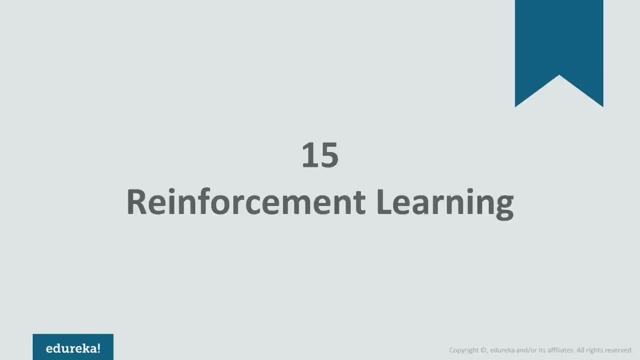 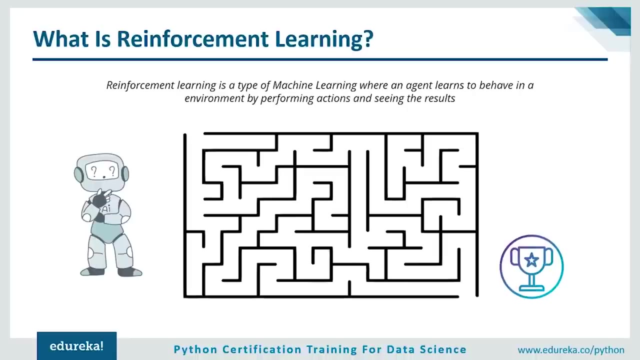 knowing what the data is, and we did clustering, different types of clustering: k-means, c-means, hierarchical clustering. three: enforcement learning is part of machine learning, where an agent is put in an environment and he learns to behave in this environment by performing certain actions. ok, so it basically performs actions and it either 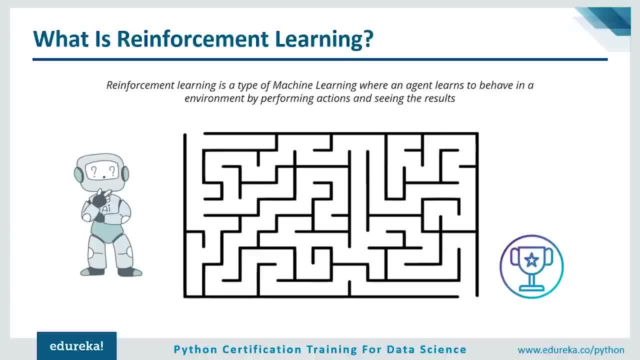 gets the rewards on the actions or it gets a punishment, and observing the reward which it gets from those actions. reinforcement learning is all about taking an appropriate action in order to maximize the reward in a particular situation. so, guys, in supervised learning, you areучi ca thai khanga. 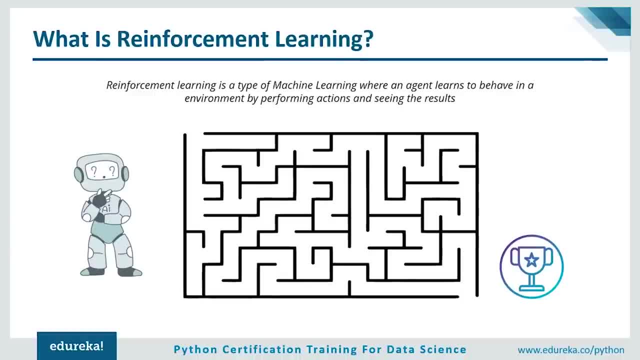 learning. the training data comprises of the input and the expected output, and so the model is trained with the expected output itself. but when it comes to reinforcement learning, there is no expected output. here the reinforcement agent decides what actions to take in order to perform a given task. in the absence of a training data set, it is bound to learn from its experience itself. 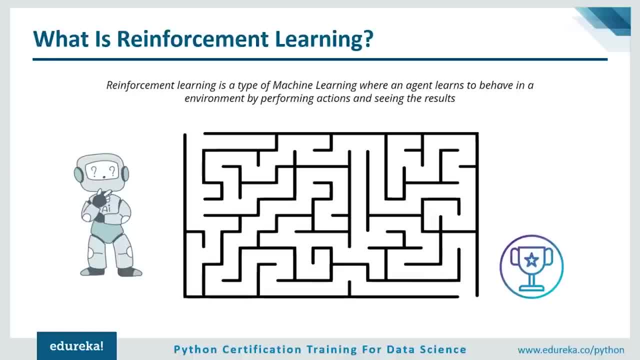 all right. so reinforcement learning is all about an agent who's put in an unknown environment and he's going to use a hit and trial method in order to figure out the environment and then come up with an outcome. okay, now let's look at reinforcement learning with an analogy. so 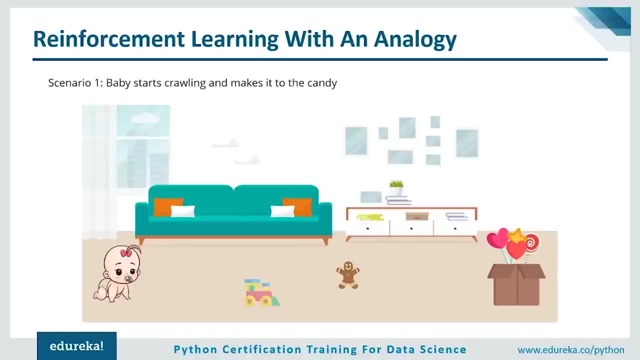 consider a scenario wherein a baby is learning how to walk. this scenario can go about in two ways now. in the first case, the baby starts walking and makes it to the candy. here, the candy is basically the reward it's going to get. so, since the candy is the end goal, the baby is happy. it's positive. 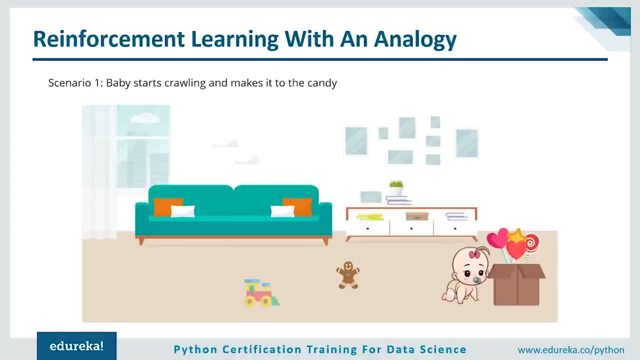 okay, so the baby is happy and it gets rewarded a set of candies. now, another way in which this could go is that the baby starts walking but falls due to some hurdle in between. the baby gets hurt and it doesn't get any candy, and obviously, the baby 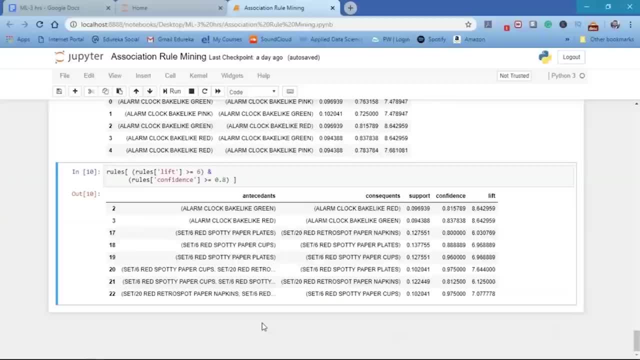 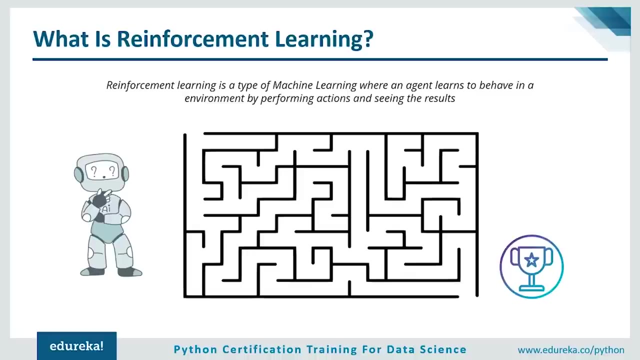 All we did was create some rules and not knowing what the data is, and we did clusterings, different types of clusterings. K means C means All right, kill class ring. Reinforcement learning is a part of machine learning, where an agent is put in an environment. 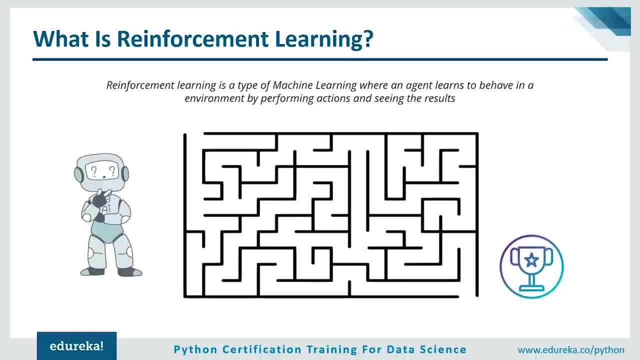 and he learns to behave in this environment by performing certain actions. Okay, so it basically performs actions and it either gets the rewards on the actions or it gets a punishment. and observing the reward which it gets from those actions, reinforcement learning is all about taking an appropriate action in order to maximize the reward. 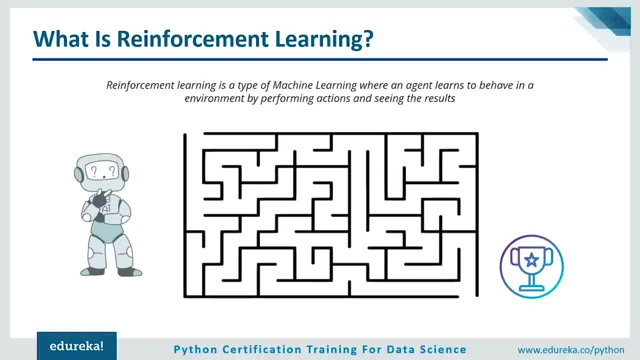 In a particular situation. So, guys, in supervised learning, the training data comprises of the input and the expected output, and so the model is trained with the expected output itself. but when it comes to reinforcement learning, there is no expected output. here The reinforcement agent decides what actions to take in order to perform a given task. in 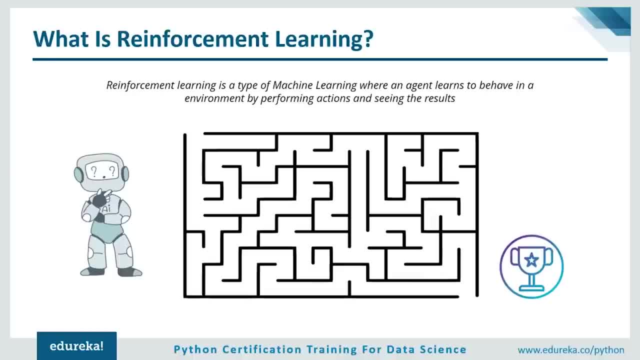 the absence of a training data set, It is bound to learn from its experience itself. All right, so reinforcement learning is all about an agent who's put in an unknown environment And he's going to use a hit and trial method in order to figure out the environment, and 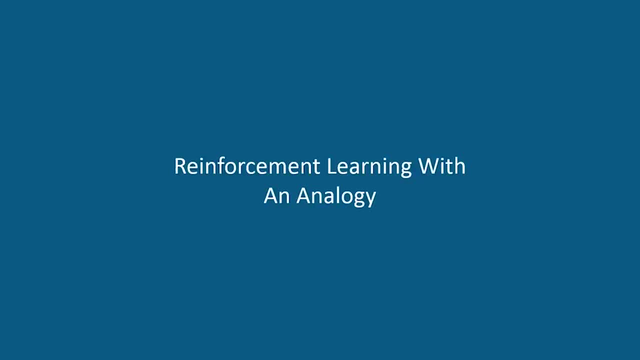 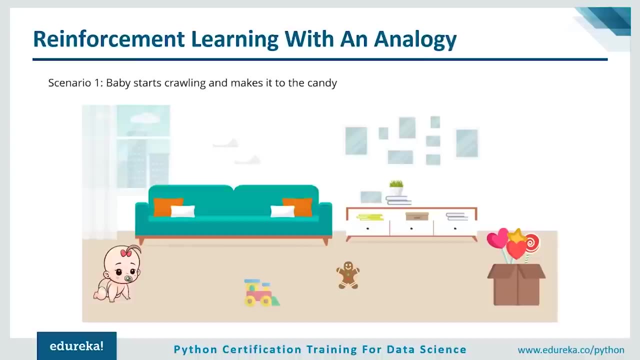 then come up with an outcome. Okay, Now let's look at reinforcement learning with an analogy. So consider a scenario wherein a baby is learning how to walk. this scenario can go about in two ways now. in the first case, the baby starts walking and makes it to the candy here. 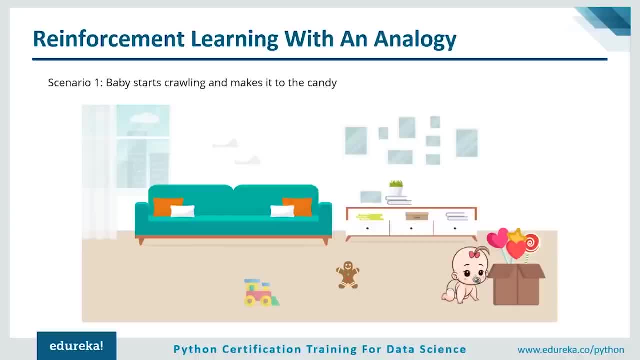 The candy is basically the reward It's going to get. so, since the candy is the end goal, the baby is happy, It's positive. Okay, so the baby is happy and it gets rewarded a set of candy. Now, another way in which this could go is that the baby starts walking but falls due to some hurdle. 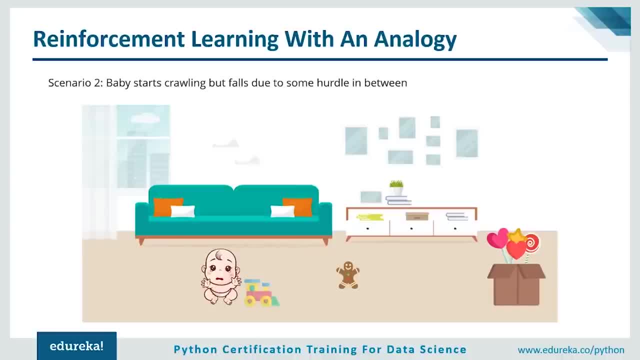 in between, the baby gets hurt and it doesn't get any candy and obviously the baby is sad. So this is a negative reward, Okay. or you can say this is a setback. So, just like how we humans learn from our mistakes by trial and error, reinforcement learning is also. 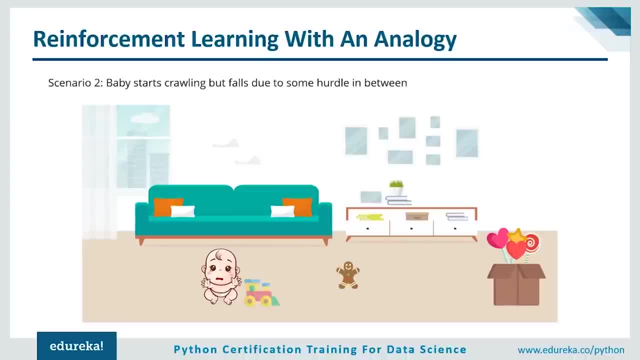 similar. Okay, So we have an agent which is basically the baby and a reward which is the candy over here. Okay, and with many hurdles in between, the agent is Suppose to find the best possible path to reach the reward. So, guys, I hope you all are clear with the reinforcement learning. 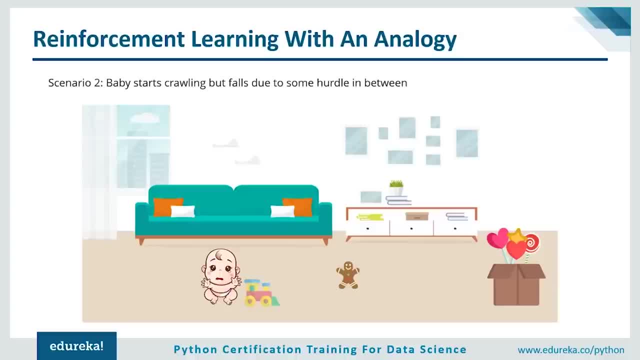 is sad. so this is a negative reward, okay. or you can say this is a setback. so, just like how we humans learn from our mistakes by trial and error, reinforcement learning is also similar, okay. so we have an agent which is basically the baby and a reward which is the candy over here. okay, and with. 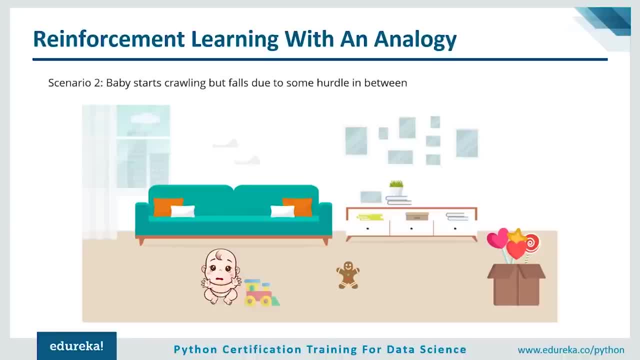 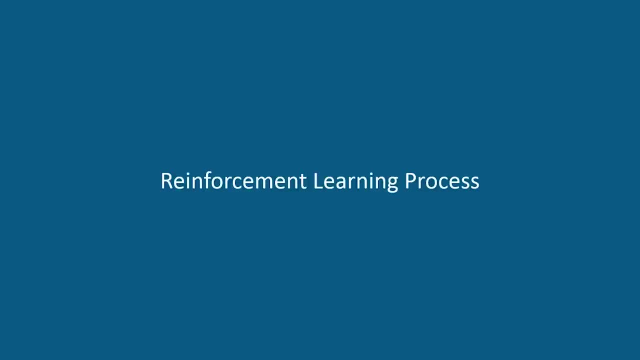 many hurdles in between. the agent is going to be the one who's going to get the candy, and the agent is supposed to find the best possible path to reach the reward. so, guys, i hope you all are clear with the reinforcement learning. now let's look at the reinforcement learning process. so 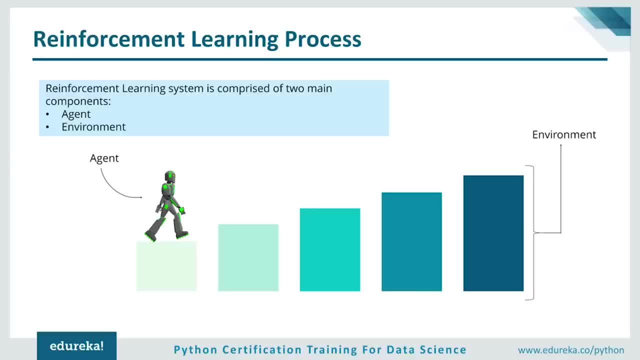 generally, a reinforcement learning system has two main components. all right, the first is an agent and the second one is an environment. now, in the previous case, we saw that the agent was a baby and the environment was the living room wherein the baby was crawling. okay, the environment is. 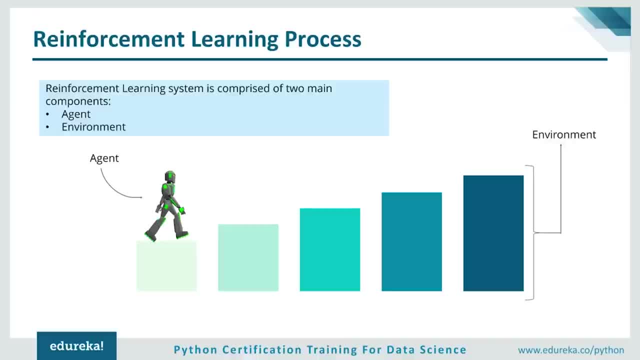 the setting that the agent is acting on, and the agent over here represents the environment, and the environment is the setting that the agent is acting on: the reinforcement learning algorithm. So, guys, the reinforcement learning process starts when the environment sends a state to the agent, and then the agent will take some actions based on. 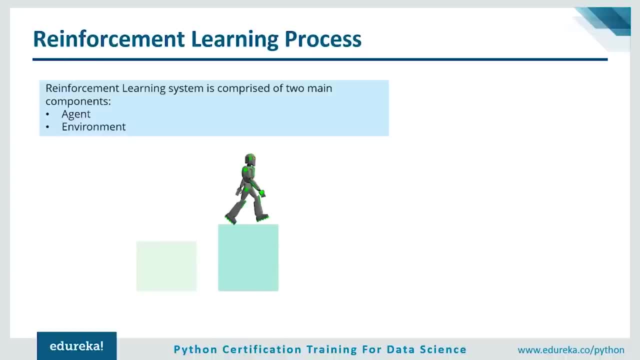 the observations. In turn, the environment will send the next state and the respective reward back to the agent. The agent will update its knowledge with a reward returned by the environment, and it uses that to evaluate its previous action. So, guys, this loop keeps continuing until the. 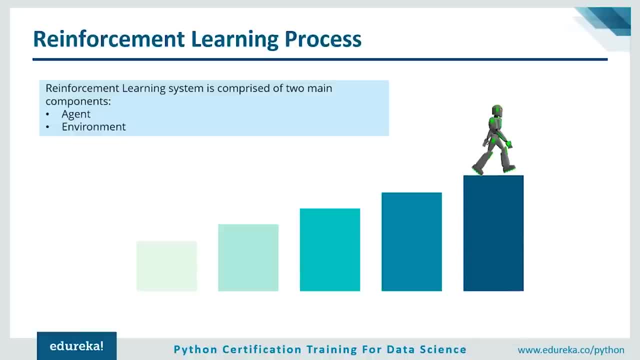 environment sends a terminal state, which means that the agent has accomplished all his tasks and he finally gets the reward. Okay, this is exactly what was depicted in this scenario. So the agent keeps climbing up ladders until he reaches his reward. To understand this better, 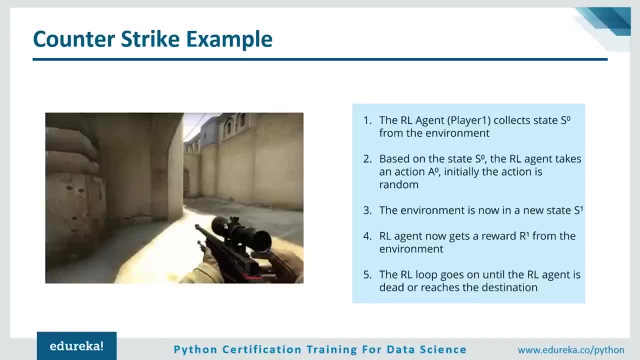 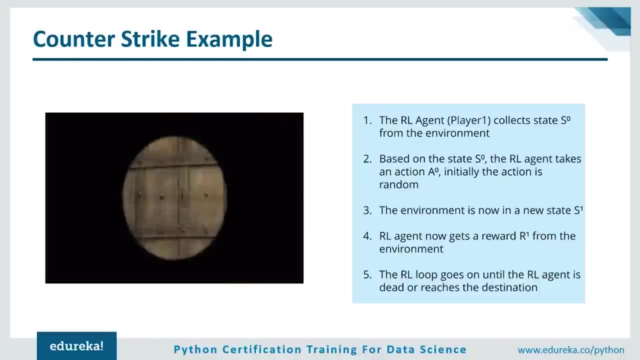 let's suppose that our agent is learning to play Counter-Strike. Okay, so let's break it down Now. initially, the RL agent, which is basically the player, player one. let's say it's the player one who is trying to learn how to play the game. Okay, he collects some state from the 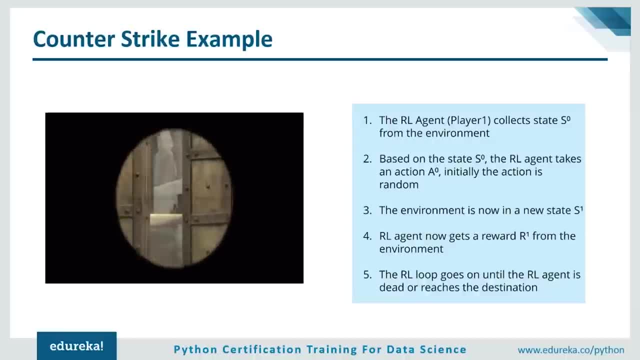 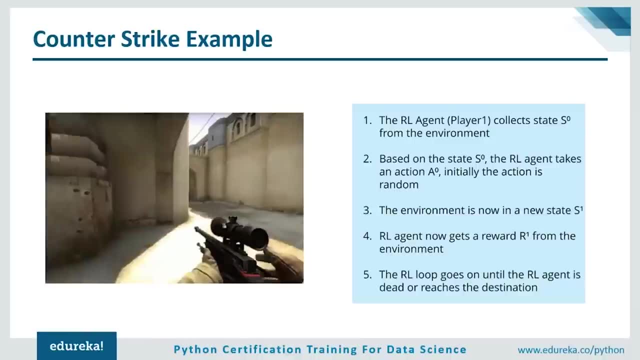 environment. Okay, this could be the first state of Counter-Strike Now, based on this state, the agent will take some action. Okay, and this action can be anything that causes a result. So if the player moves left or right, it's also considered as an action. Okay, so initially, 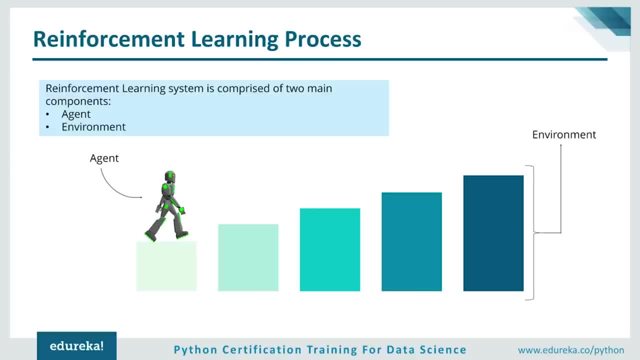 Now let's look at the reinforcement learning process. So, generally, a reinforcement learning system has two main components. All right, The first is an agent and the second one is an environment. Now, in the previous case, we saw that the agent was a baby and the environment was the living room. 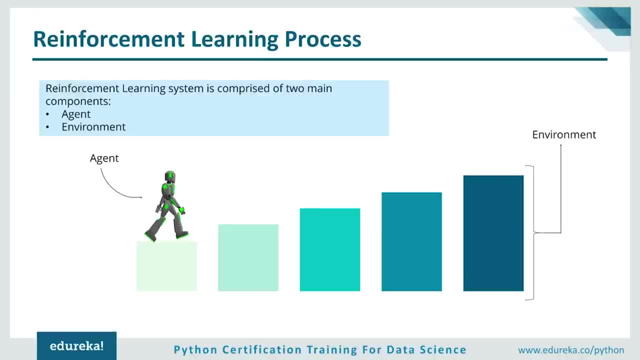 where in the baby was crawling. Okay, the environment is the setting that the agent is acting on, and the agent over here represents the reinforcement learning algorithm. So, guys, the reinforcement learning process starts when the environment sends a state to the agent, and then the agent will take some actions based on the observations in turn, 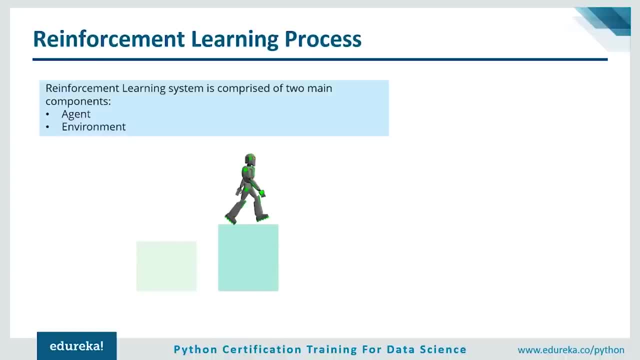 The environment will send the next state and the respective reward back to the agent. The agent will update its knowledge with a reward returned by the environment, and it uses that to evaluate its previous action. So, guys, this loop keeps continuing until the environment sends a terminal state, which means that 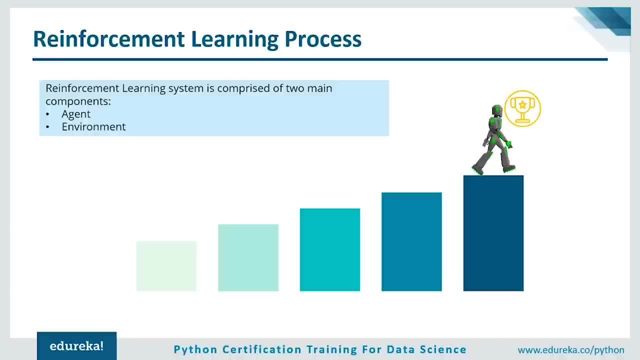 the agent has accomplished all his tasks and he finally gets the reward. Okay, this is exactly what was depicted in this scenario. So the agent keeps climbing up ladders until he reaches his reward. to understand this better, Let's suppose that our agent is learning to play counter-strike. 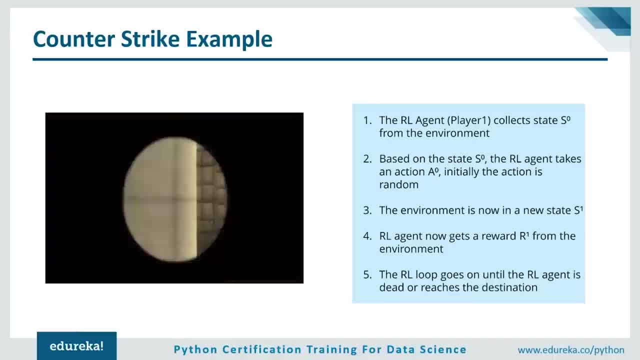 Okay, so let's break it down now. initially, the RL agent, which is basically the player- player one, Let's say, it's the player one who is trying to learn how to play the game. Okay, he collects some state from the environment. Okay, this could be the first state of counter-strike. 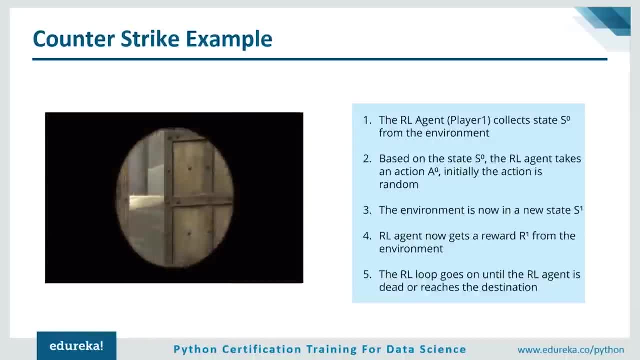 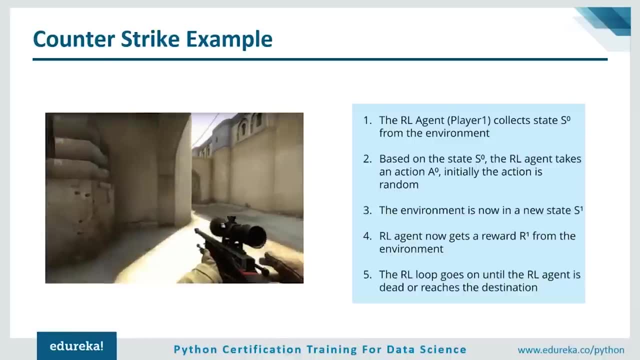 Now, based on the state, the agent will take some action. Okay, and this action can be anything that causes a result. So if the player moves left or right, it's also considered as an action Okay. So initially the action is going to be random because obviously the first time you pick up counter-strike- 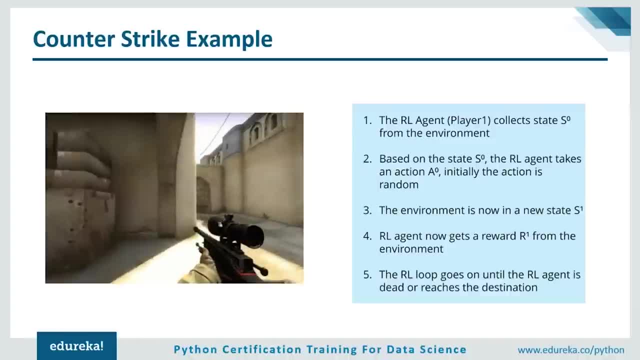 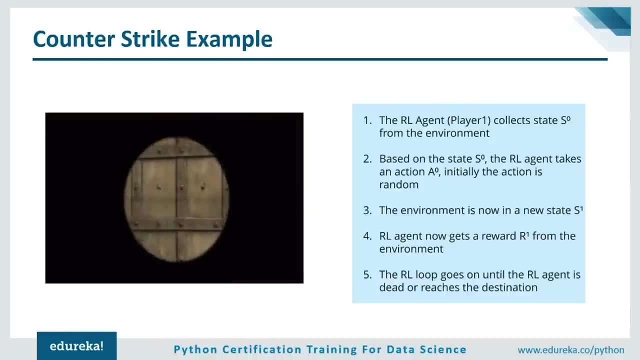 you're not going to be a master at it, So you're going to try with different actions and you're just going to pick up a random action in the beginning. Now the environment is going to give a new state. So, after clearing that, the environment is now going to give a new state to the agent or to the player. 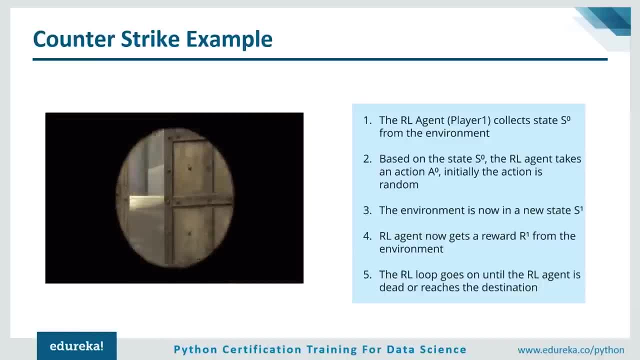 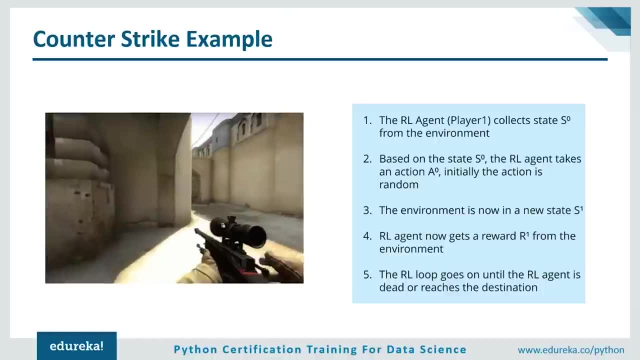 So maybe he's cross stage one now He's in stage two. So now the player will get a reward- R1- from the environment because it cleared stage one. So this reward can be anything. it can be additional points or coins or anything like that. 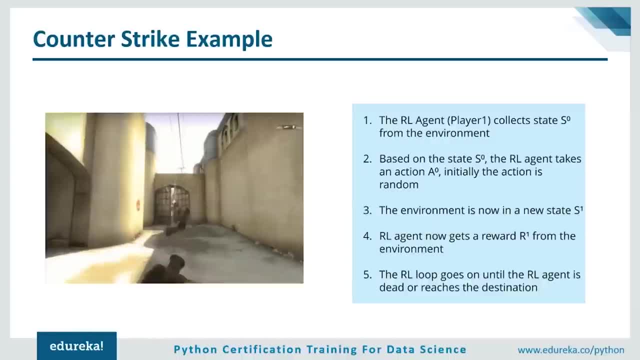 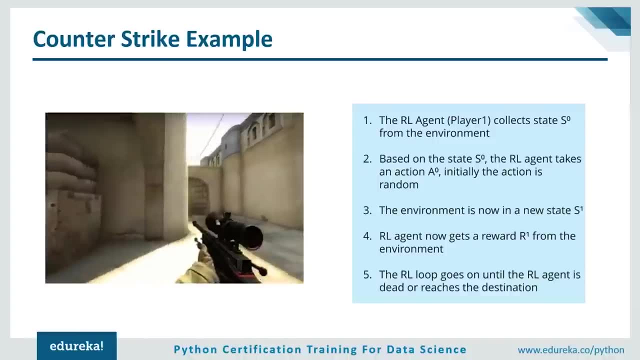 the action is going to be random because obviously the first time you pick up Counter-Strike you're not going to be a master at it, So you're going to try with different actions and you're just going to pick up a random action in the beginning. Now the environment is going to give. 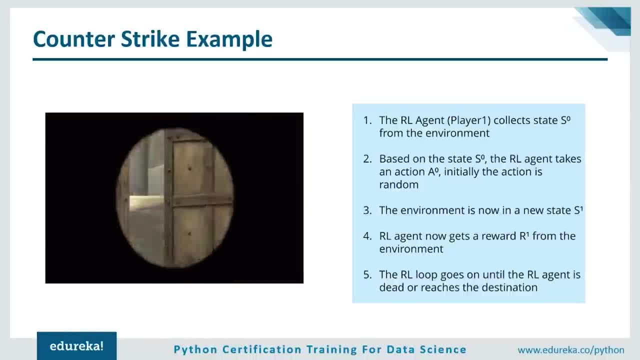 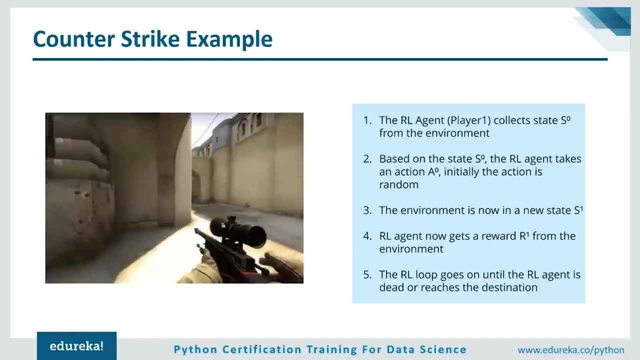 a new state. So after clearing that, the environment is now going to give a new state to the agent or to the player. So maybe he's across stage one Now he's in stage two. So now the player will get a reward R1- from the environment because it 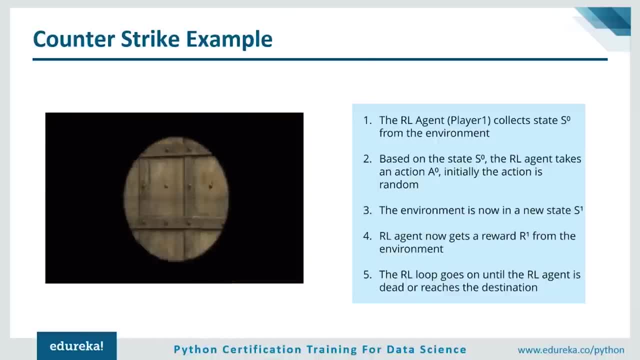 cleared stage one. So this reward can be anything. It can be additional points or coins or anything like that, Okay. so basically, this loop keeps going on until the player is dead or reaches the destination- Okay, and it continuously outputs a sequence of states, actions and rewards. So, guys, this was a small example to show you how to clear a reward. So let's go ahead and let's see how to clear a reward. So let's go ahead and let's see how to clear a reward. So let's go ahead and let's see how. 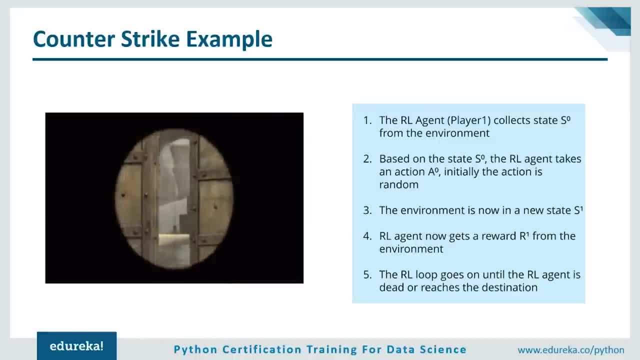 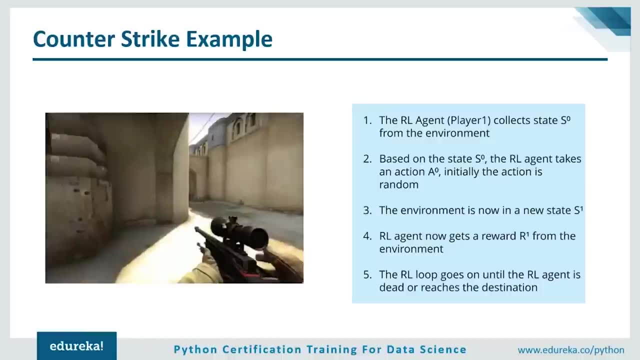 reinforcement learning process works. So you start with an initial state and once the player clears that state, he gets a reward. After that, the environment will give another stage to the player and after it clears that state, it's going to get another reward and it's going to keep. 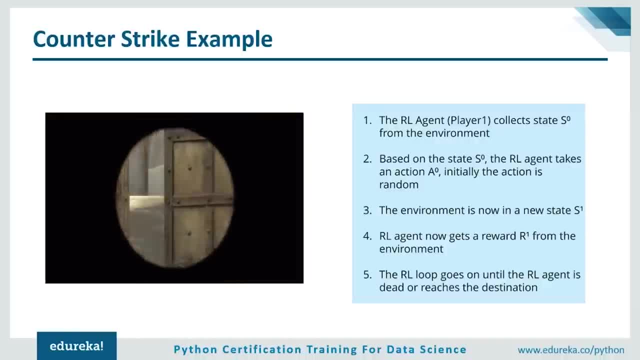 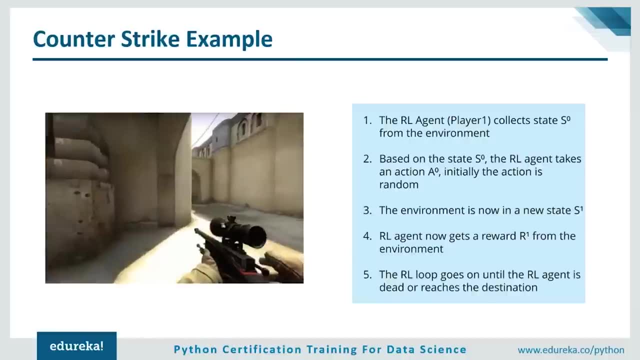 happening until the player reaches his destination. All right. so, guys, I hope this is clear. Now let's move on and look at the reinforcement learning definitions. So there are a few concepts that you should be aware of while studying reinforcement learning. Let's look at those. 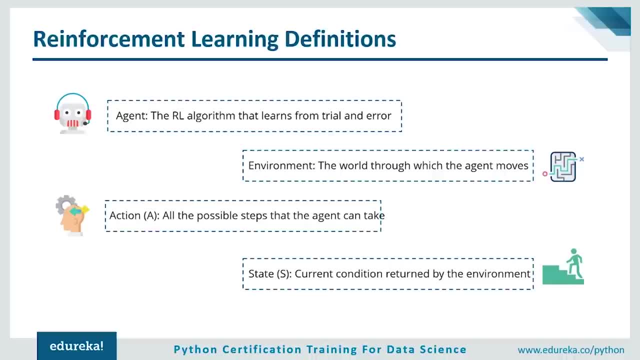 definitions over here. So first we have the agent. Now. an agent is basically the reinforcement learning algorithm that learns from trial and error. Okay, so an agent takes actions like, for example, a soldier in Counter-Strike navigating through the game. that's also an action, Okay. 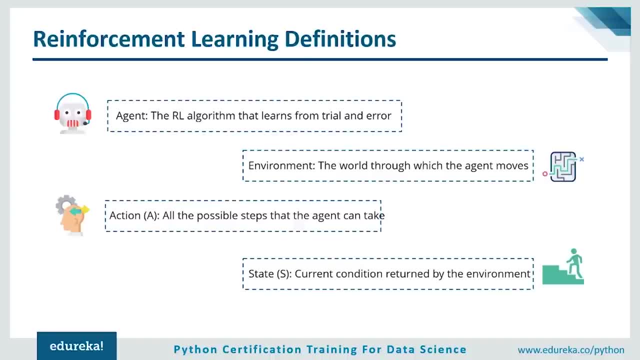 if he moves left, right or if he shoots at somebody, that's also an action. Okay, so the agent is responsible for taking actions in the environment. Now, the environment is the whole Counter-Strike game. Okay, it's basically the world through which the agent moves. The 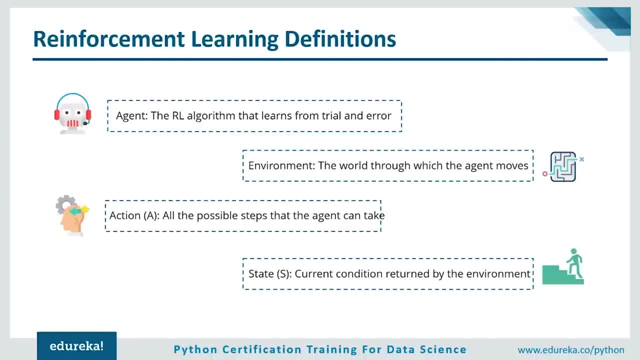 environment takes the agent's current state and action as input and it returns the agent's reward and its next state as output. All right, Next we have action. Now all the possible steps that an agent can take are called actions. So, like I said, it can be moving right, left or shooting, or any. 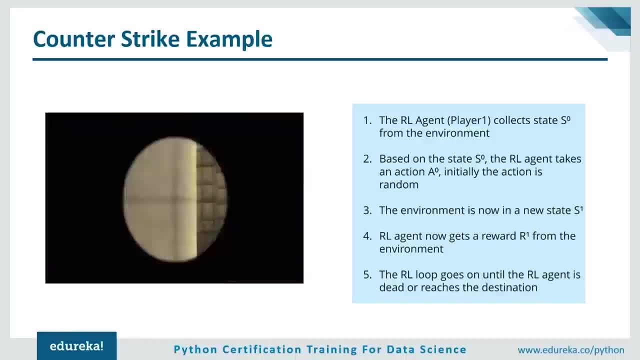 Okay. So, basically, this loop keeps going on until the player is dead or reaches the destination- Okay, and it continuously outputs a sequence of states, actions and rewards. So, guys, this was a small example to show you how reinforcement learning process works. So you start with this. 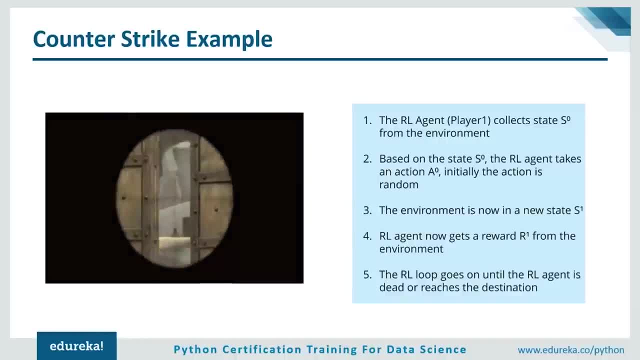 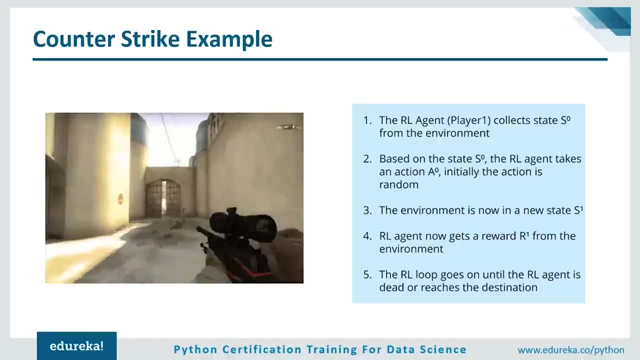 Start with an initial state and once the player clears that state, he gets a reward. after that, the environment will give another stage to the player and after it clears that state, it's going to get another reward. and it's going to keep happening until the player reaches his destination. 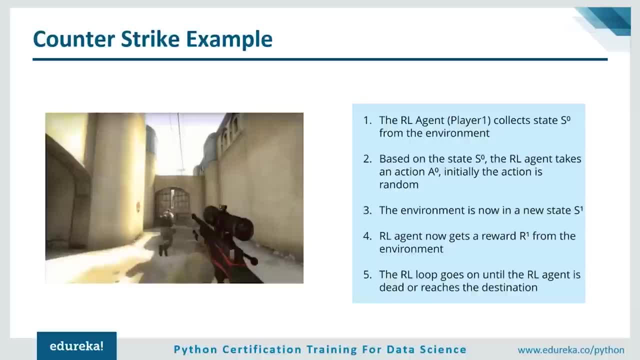 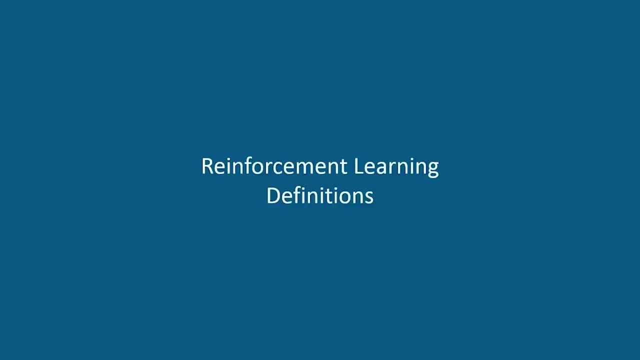 All right. So, guys, I hope this is clear. Now let's move on and look at the reinforcement learning definitions. So there are a few concepts that you should be aware of while studying reinforcement learning. Let's look at those definitions over here. 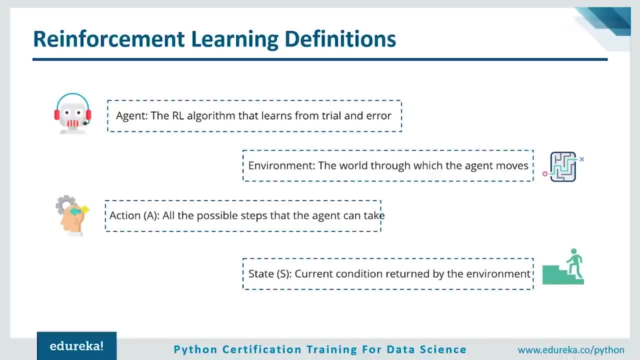 So first we have the agent. Now an agent is basically the reinforcement learning algorithm that learns from trial and error. Okay, So an agent takes actions like, for example, a soldier in counter-strike navigating through the game. That's also an action. 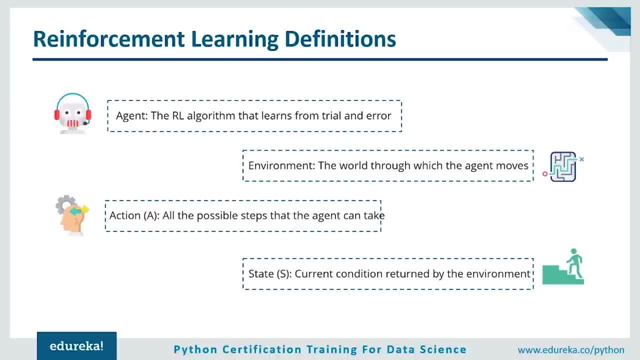 Okay, if he moves left, right or if he shoots at somebody, that's also an action. Okay, So the agent is responsible for taking actions in the environment. Now, the environment is the whole counter-strike game. Okay, it's basically the world through which the agent moves. the environment takes the. 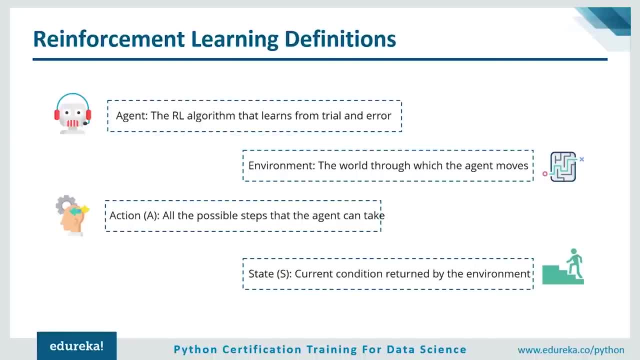 agents current state and action as input And it returns the agents reward and its next state as output. All right, Next we have action. now all the possible steps that an agent can take are called actions. So, like I said, it can be moving right, left or shooting or any of that. 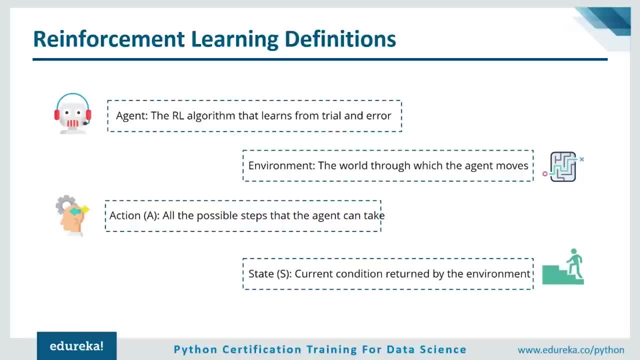 All right, then we have state. now, state is basically the current condition returned by the environment. So, whichever state you are in, if you are in state 1 or if you're in state 2, that represents your current condition, All right. Next, we have reward. 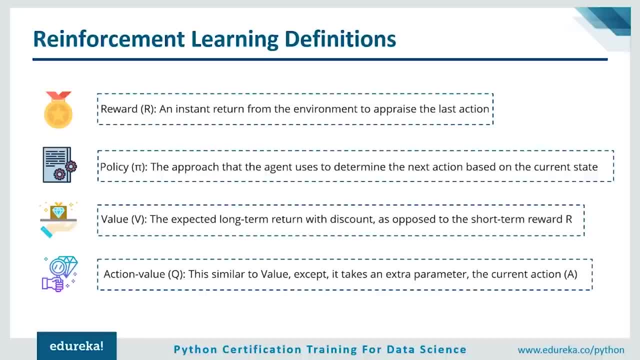 A reward is basically an instant return from the environment to appraise your last action. Okay, so it can be anything like coins or it can be additional points. So basically, a reward is given to an agent after it clears the specific stages. next we have policy. policy is basically the strategy that the agent uses to find out his next action. 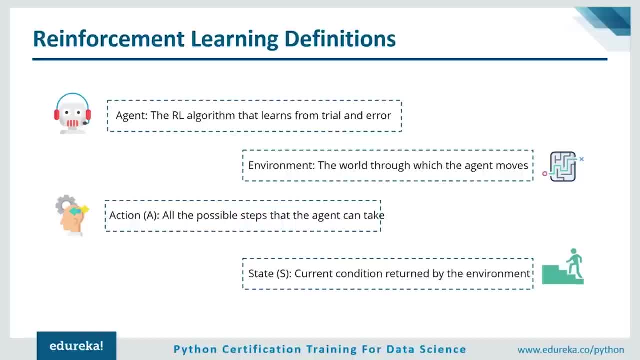 of that. All right, then we have state. Now, state is basically the current condition returned by the environment. So, whichever state you are in, if you're in state one or if you're in state two, that represents your current condition. 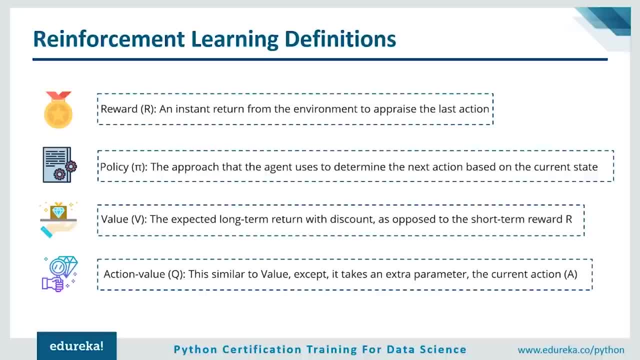 All right. Next we have reward. A reward is basically an instant return from the environment to appraise your last action. Okay, so it can be anything like coins or it can be additional points. So basically, a reward is given to an agent after it clears the specific stages. Next, 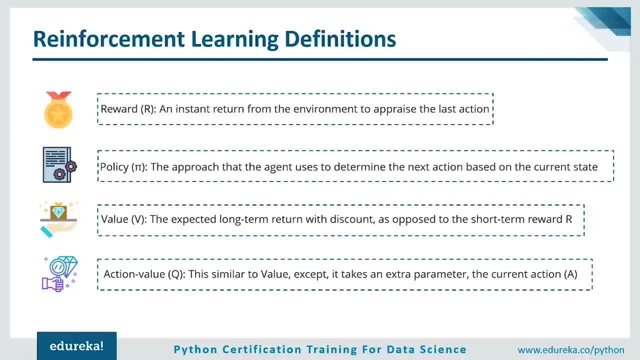 we have policy. Policy is basically the strategy that the agent uses to find out his next action based on his current state. Policy is just the strategy with which you approach the game. Then we have value. Now value is the expected long-term return with discount. So value and action value. 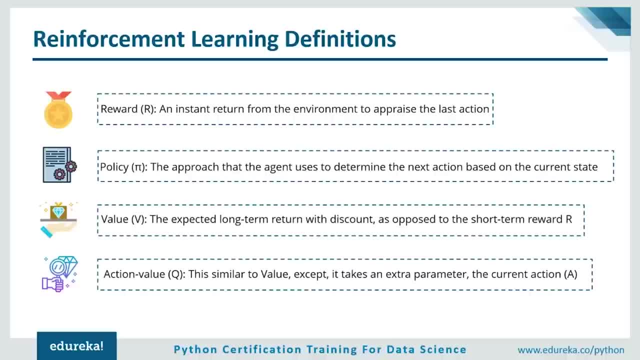 can be a little bit confusing for you right now, but as we move further you'll understand what I'm talking about. Okay, so value is basically the long-term return that you get with discount. Okay, discount I'll explain in the further slides. Then we have action value. Now action value is: 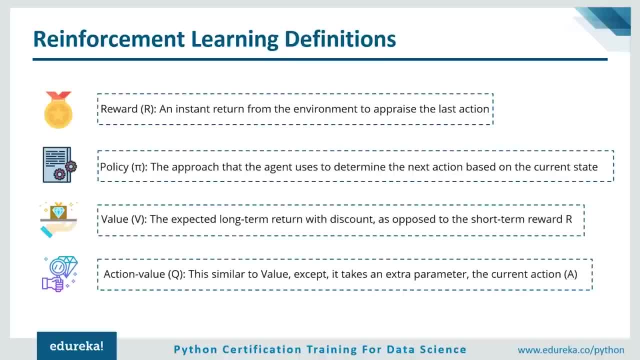 also known as Q value. Okay, it's very similar to value, except that it takes an extra parameter, which is the current action. So, basically, here you'll find out the Q value, depending on the particular action that you took. All right, So, guys, don't get confused. 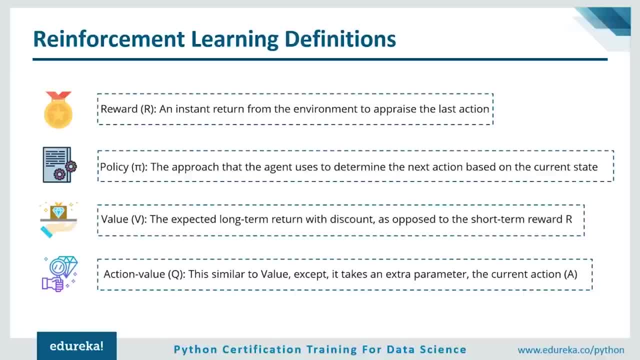 with value and action value. We look at examples in the further slides and you'll understand this better. Okay, so, guys, make sure that you're familiar with these terms, because you'll be seeing a lot of these terms in the further slides. All right Now, before we move any further. 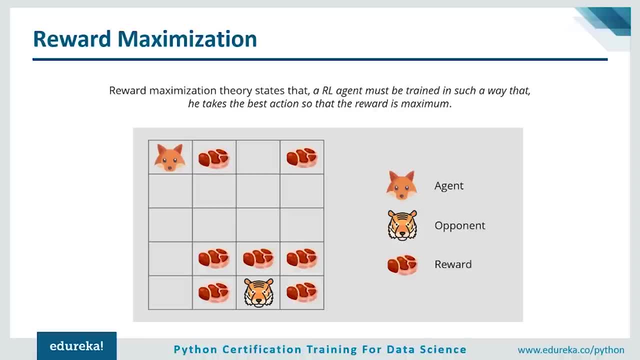 I'd like to discuss a few more concepts. Okay, so first we'll discuss the reward maximization. So, if you haven't already realized it, the basic aim of the RL agent is to maximize the reward. So, if you haven't already realized it, the basic aim of the RL agent is to 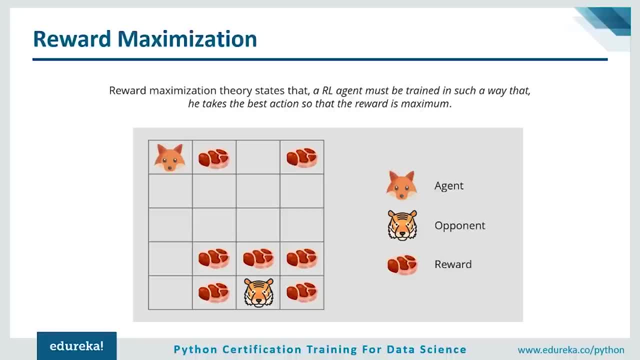 maximize the reward. So, if you haven't already realized it, the basic aim of the RL agent is to maximize the reward. Now, how does that happen? Let's try to understand this in depth. So the agent must be trained in such a way that he takes the best action so that the reward is maximum. 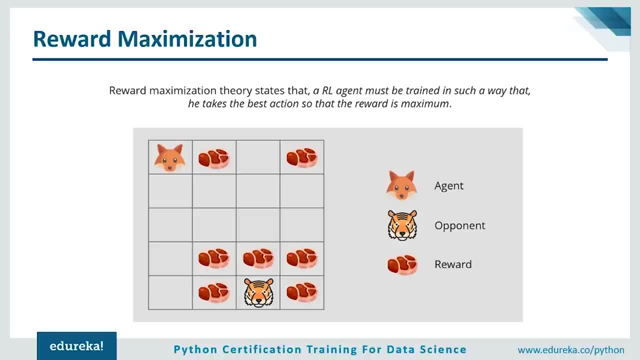 because the end goal of reinforcement learning is to maximize your reward based on a set of actions. So let me explain this with a small game. Now. in the figure you can see there is a fox, there's some meat and there's a tiger. So our agent is basically the fox and his end goal is: 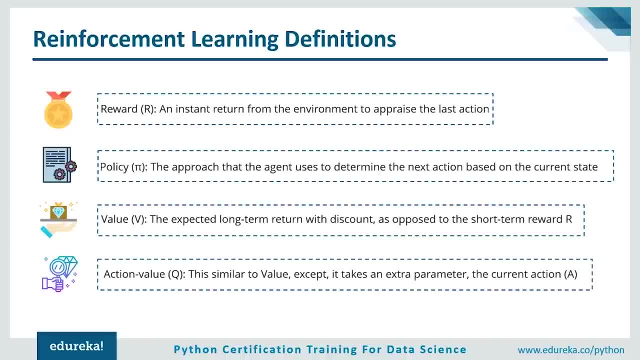 based on his current state policy is just the strategy with which you approach the game. Then we have value. now. Value is the expectation. It long-term return with discount. So value and action value can be a little bit confusing for you right now. 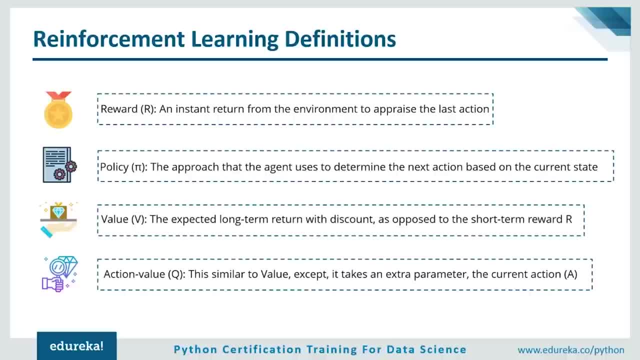 But as we move further, you'll understand what I'm talking about. Okay, So value is basically the long-term return that you get with discount. Okay, discount I'll explain in the further slides. Then we have action value now. action value is also known as Q value. 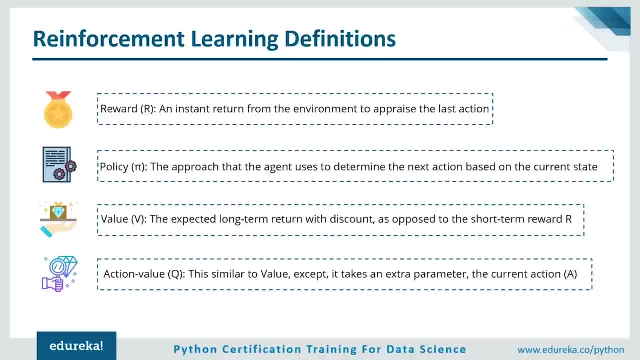 Okay, It's very similar to value, except that it takes an extra parameter, which is the current action. So basically, here you'll find out the Q value, depending on the particular action That you took. All right, so guys don't get confused with value and action value. 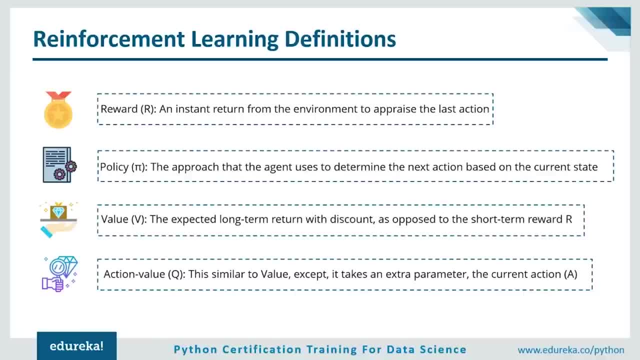 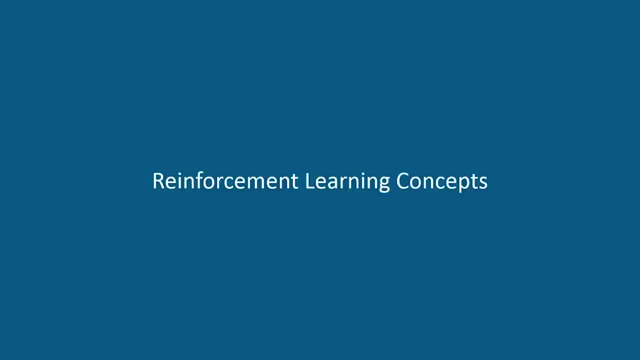 We look at examples in the further slides and you'll understand this better. Okay, so, guys, make sure that you're familiar with these terms, because you'll be seeing a lot of these terms in the further slides. All right now, before we move any further. 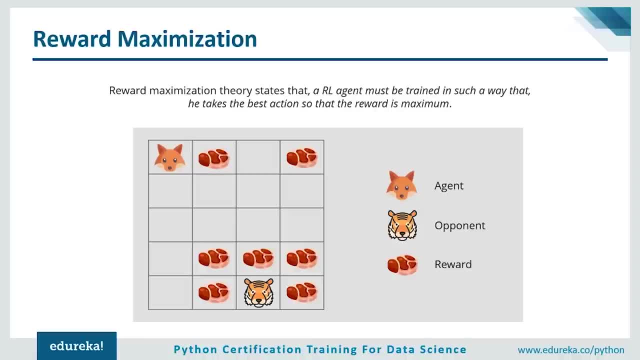 I'd like to discuss a few more concepts. Okay, So first we'll discuss the reward maximization. So, if you haven't already realized it, the basic aim of the RL agent is to maximize the reward. Now, how does that happen? Let's try to understand this in depth. 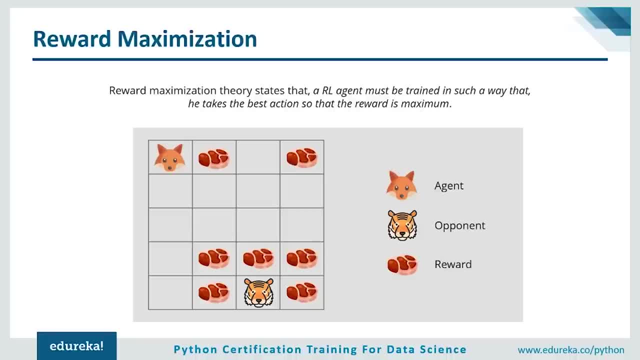 So the agent must be trained in such a way that he takes the best action so that the reward is maximum, because the end goal of reinforcement learning is to maximize your reward based on a set of actions. So let me explain this with a small game. 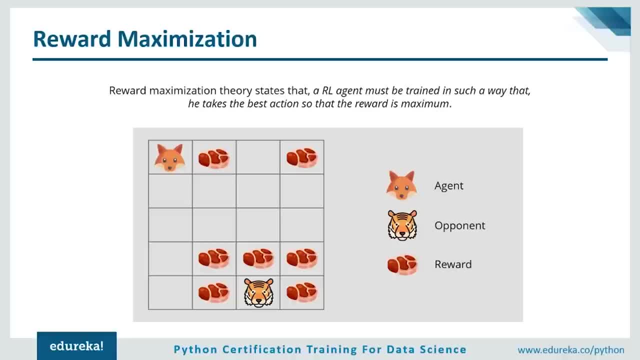 Now in the figure you can see there is a fox, There's some meat and there's a tiger. So our agent is basically the Fox and his end goal is to eat the maximum amount of meat before being eaten by the tiger. Now, since the fox, 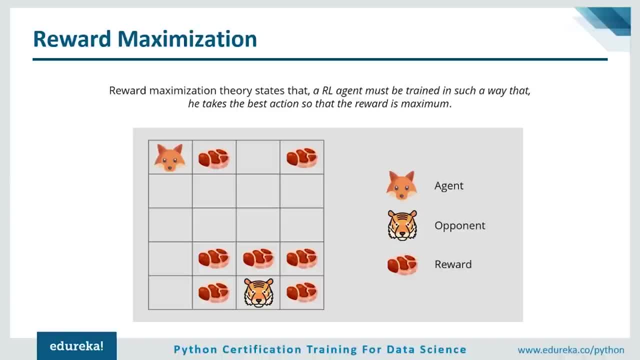 Is a clever fellow. He eats the meat that is closer to him rather than the meat which is closer to the tiger. Now, this is because the closer he is to the tiger, the higher are his chances of getting killed. So, because of this, the rewards which are near the tiger, even if they are bigger meat chunks. 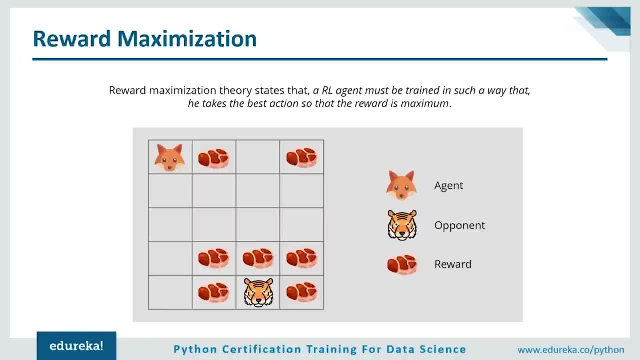 they will be discounted. So this is exactly what discounting means. So our agent is not going to eat the meat chunks which are closer to the tiger because of the risk. All right Now, even though the meat chunks might be larger, he does not want to take the chances of getting killed. 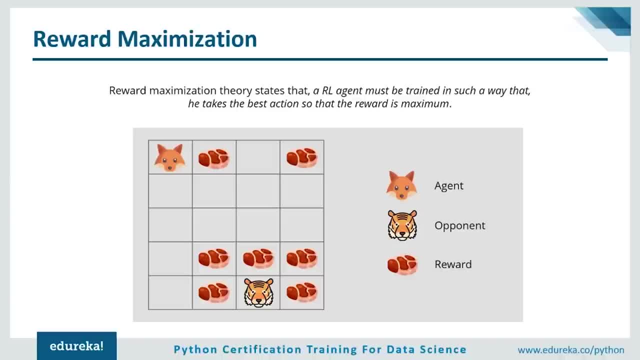 to eat the maximum amount of meat before being able to eat the rest of the food. So let's start being eaten by the tiger Now. since the fox is a clever fellow, he eats the meat that is closer to him, rather than the meat which is closer to the tiger. Now, this is because the closer he is to 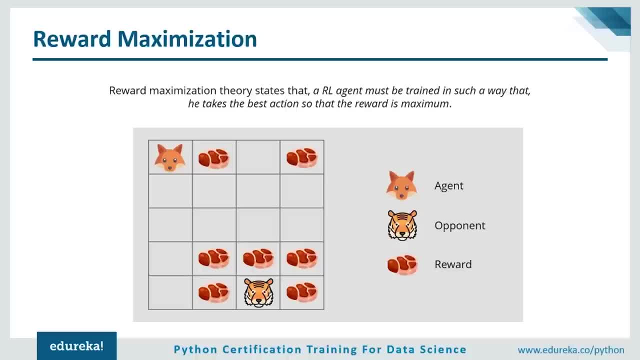 the tiger, the higher are his chances of getting killed. So, because of this, the rewards which are near the tiger, even if they are bigger meat chunks, they will be discounted. So this is exactly what discounting means. So our agent is not going to eat the meat chunks which are closer to the 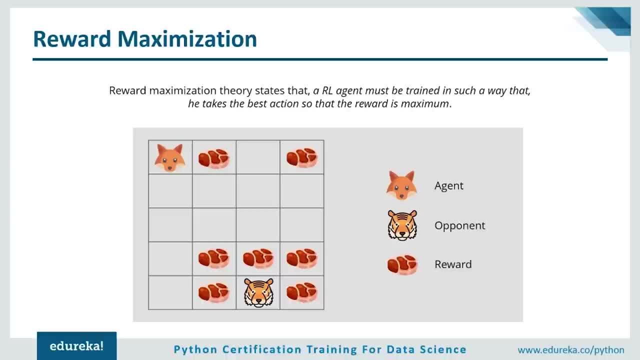 tiger because of the risk. Now, even though the meat chunks might be larger, he does not want to take the chance to eat the meat, So he is not going to eat the meat chunks which are closer to. Okay, this is called discounting. Okay, this is where you discount because you improvise and you 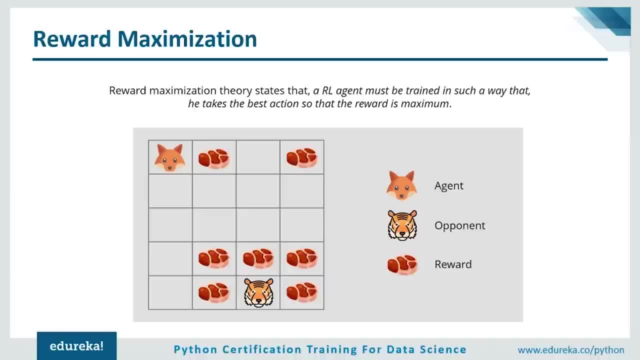 just eat the meat which are closer to you, instead of taking risks and eating the meat which are closer to your opponent. All right Now. the discounting of reward works based on a value called gamma. We'll be discussing gamma in our further slides, But, in short, the value of gamma. 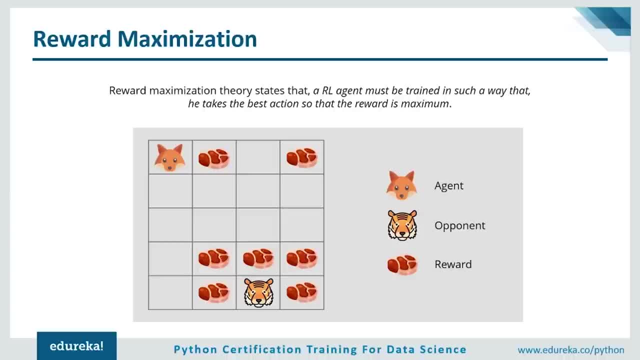 is between zero and one. Okay, so the smaller the gamma, the larger is the discount value. Okay, so if the gamma value is lesser, it means that the agent is not going to explore and he's not going to try and eat the meat chunks. 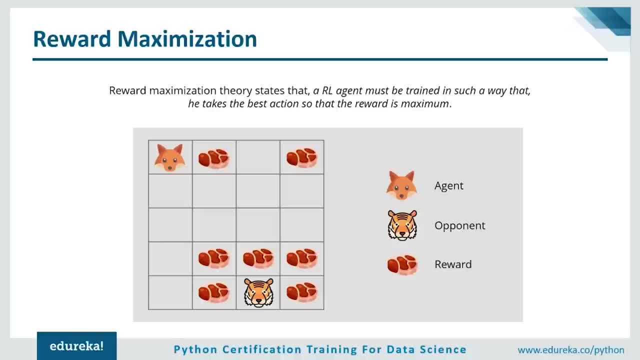 which are closer to the tiger. Okay, but if the gamma value is closer to one, it means that our agent is actually going to explore and it's going to try and eat the meat chunks which are closer to the tiger. All right, Now I'll be explaining this in depth in the further slides, So don't. 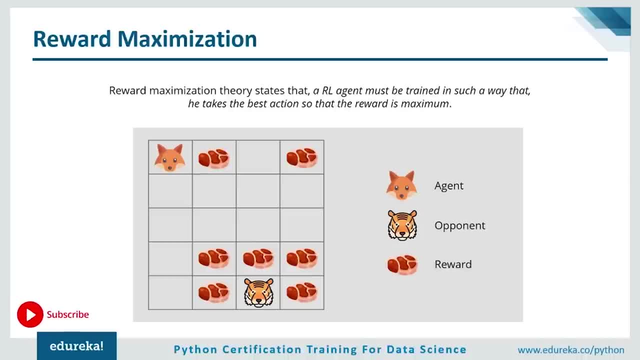 worry if you haven't got a clear concept yet, But just understand that reward maximization is a very important step when it comes to reinforcement learning, because the agent has to collect maximum rewards by the end of the game. All right, Now let's look at another concept, which is called. 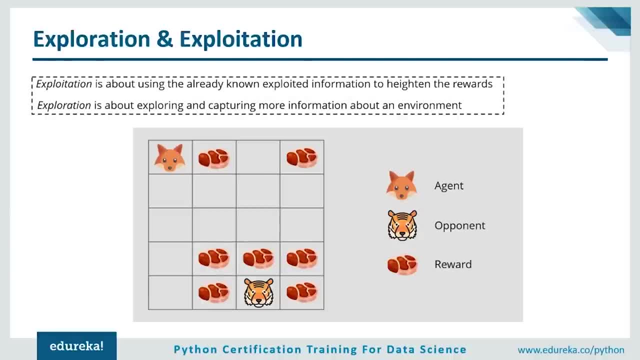 exploration and exploitation. So exploration, like the name suggests, is about exploring and capturing more information about an environment. On the other hand, exploitation is about using the already known, exploited information to heighten the rewards. So, guys, consider the fox and tiger example that we discussed Now here. the fox eats only the meat chunks which are close to him. 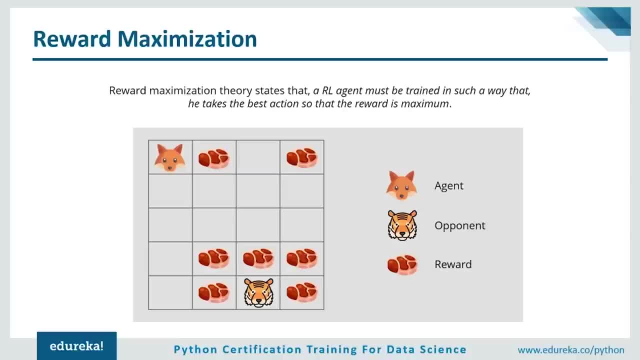 Okay, This is called discounting. Okay, This is where you discount because you improvise and you just eat the meat which are closer to you, instead of taking risks and eating the meat which are closer to your opponent. All right, Now, the discounting of reward works based on a value called gamma. 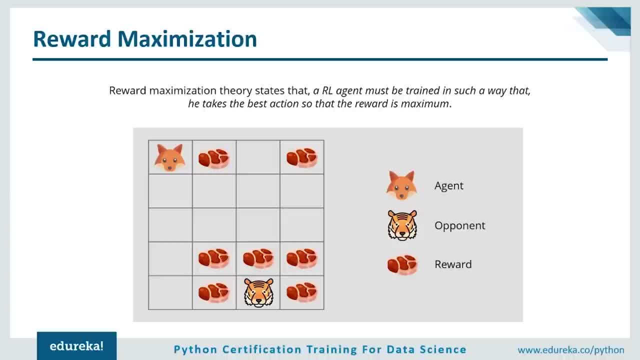 We'll be discussing gamma in our further slides, but, in short, the value of gamma is between 0 and 1.. Okay, So the smaller the gamma, the larger is the discount value. Okay, So if the gamma value is lesser, it means that the agent 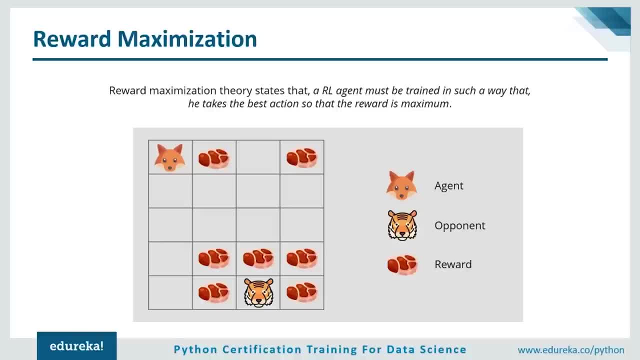 Is not going to explore and he's not going to try and eat the meat chunks which are closer to the tiger. Okay, but if the gamma value is closer to one, it means that our agent is actually going to explore and it's going to try and eat the meat chunks which are closer to the tiger. 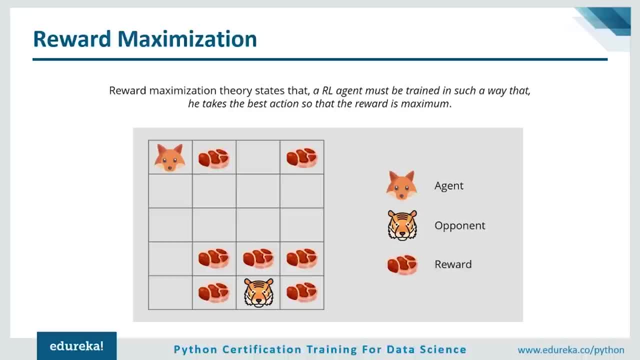 All right Now. I'll be explaining this in depth in the further slides, So don't worry if you haven't got a clear concept yet, but just understand that reward maximization is a very important step when it comes to reinforcement learning, because the agent has to collect. 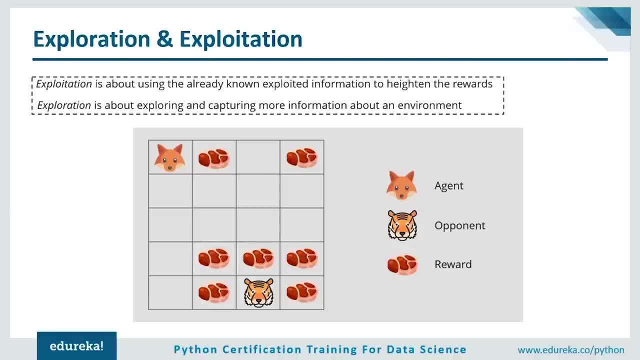 maximum rewards by the end of the game. All right, Now let's look at another concept, which is called exploration and exploitation. So exploration, like the name suggests, is about exploring and capturing more information about an environment. On the other hand, exploitation is about using the already known exploited information to heighten 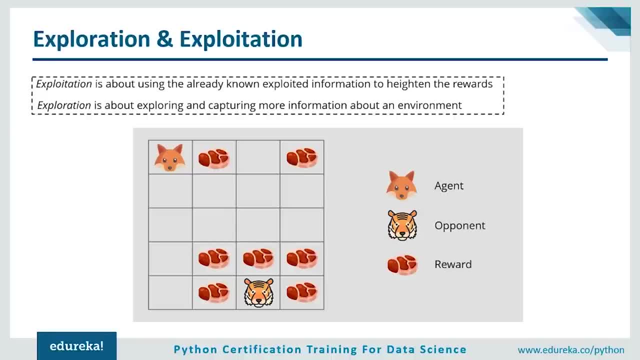 the rewards. So guys consider the fox and tiger example that we discussed now here. the Fox eats only the meat chunks which are close to him, but he does not eat the meat chunks which are closer to the tiger. Okay, even though they might give him more. 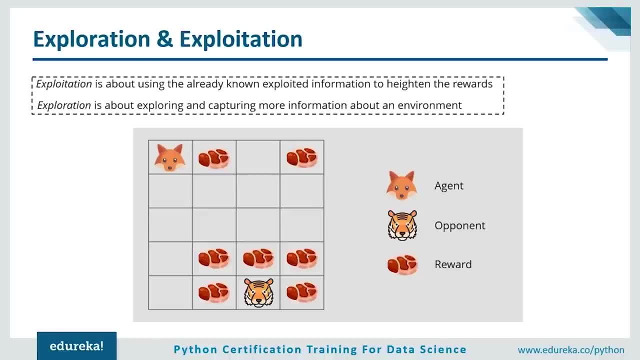 Rewards, He does not eat them. If the Fox only focuses on the closest rewards, he will never reach the big chunks of meat. Okay, This is what exploitation is about. You're just going to use the currently known information and you're going to try and get rewards based. 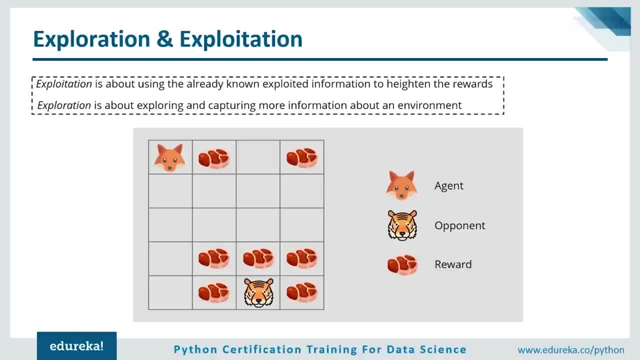 on that information. But if the Fox decides to explore a bit, it can find the bigger reward, which is the big chunks of meat. This is exactly what exploration is. So the agent is not going to stick to one corner. instead, He's going to explore the entire environment. 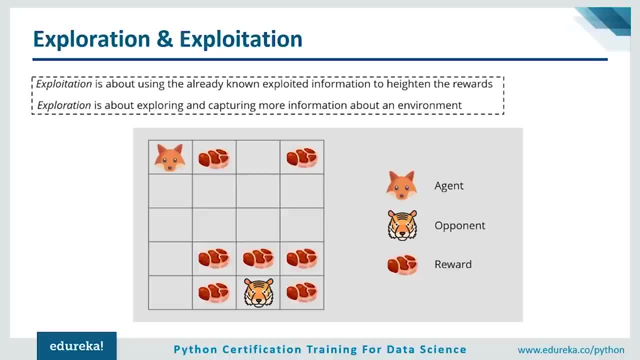 but he does not eat the meat chunks which are closer to the tiger. Okay, Even though they might give him more rewards, he does not eat them. If the fox only focuses on the closest rewards, he will never reach the big chunks of meat. Okay, This is what. 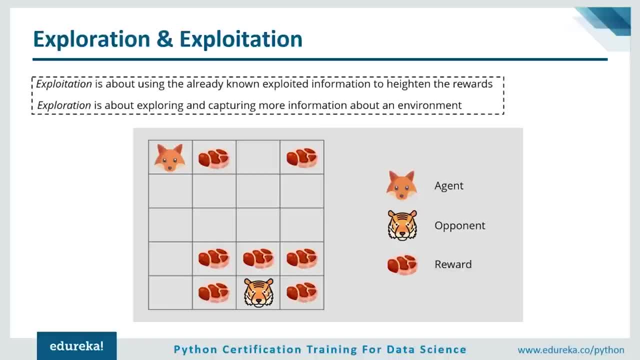 exploitation is about: You're just going to use the currently known information and you're going to try and get rewards based on that information. But if the fox decides to explore a bit, it can find the bigger reward, which is the big chunks of meat. This is exactly what exploration is. 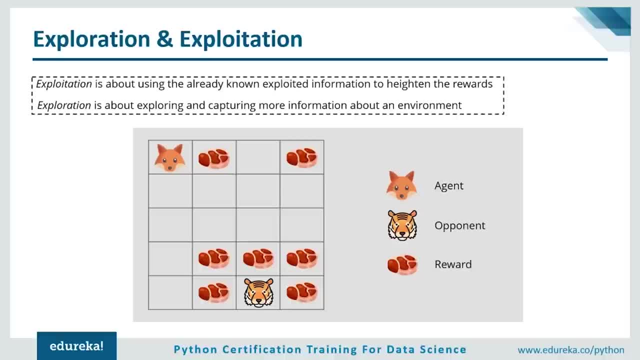 So the agent is not going to stick to one corner. Instead, he's going to explore the entire environment and try and collect bigger rewards. All right, So, guys, I hope you all are clear with exploration and exploitation. Now let's look at the 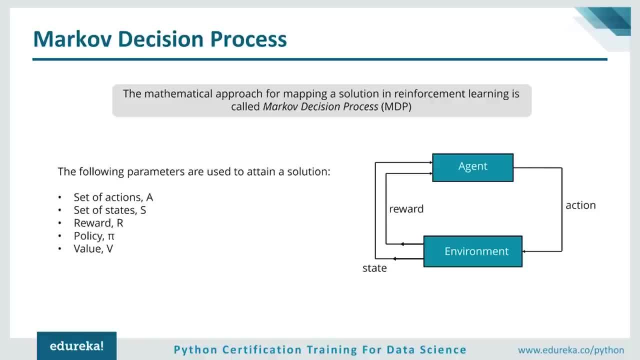 Markov's decision process. So, guys, this is basically a mathematical approach for mapping a solution in reinforcement learning. In a way, the purpose of reinforcement learning is to solve a Markov decision process. Okay, So there are a few parameters that are used to get to the solution. 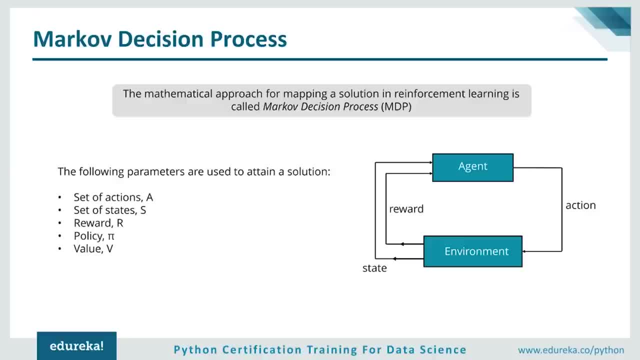 So the parameters include the set of actions, the set of states, the rewards, the policy that you're taking to approach the problem and the value that you get. Okay, So, to sum it up, the agent must take an action A to transition from 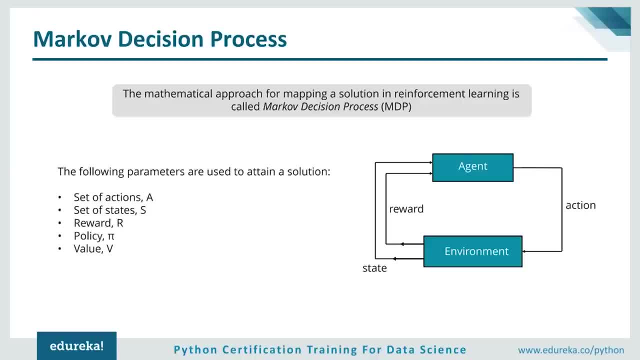 a start state to the end state S. While doing so, the agent will receive a reward R for each action that he takes. So, guys, a series of actions taken by the agent define the policy, or it defines the approach, and the rewards that are collected define the value. So the main goal here is to 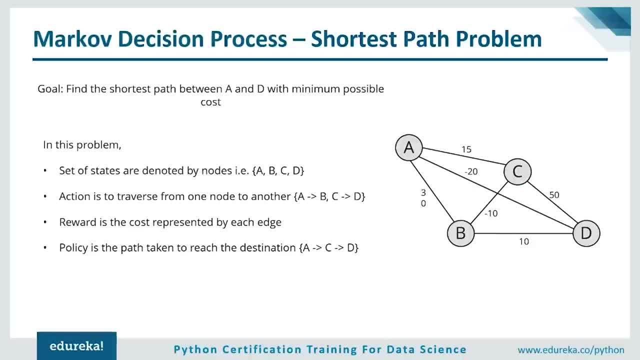 maximize the rewards by choosing the optimum policy. All right, Now let's try to understand this with the help of the shortest path problem. I'm sure a lot of you might have gone through this problem when you were in college. So, guys, look at the graph over here. So our aim here is to find 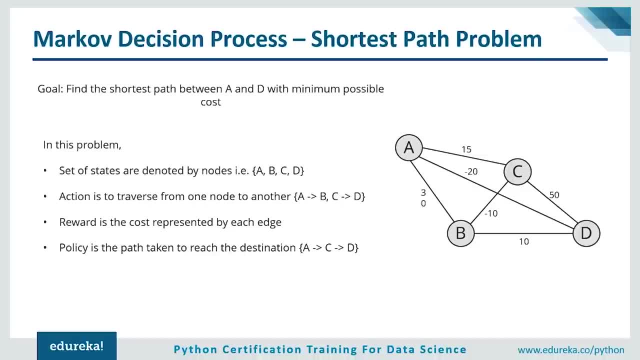 the shortest path between A and D with minimum possible cost. So the value that you see on each of these edges basically denotes the cost. So if I want to go from A to C, it's going to cost me 15 points, Okay, So let's look at how this is going to work. So let's look at the graph over here. 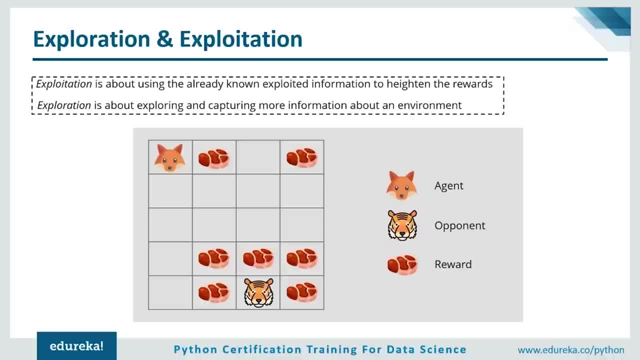 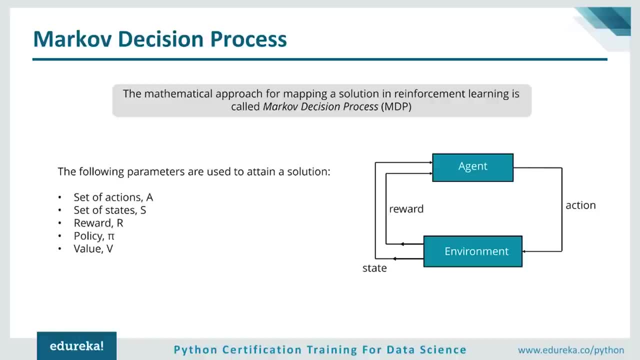 And try and collect bigger rewards. All right, So, guys, I hope you all are clear with exploration and exploitation. Now let's look at the markers decision process. So, guys, this is basically a mathematical approach for mapping a solution in reinforcement learning. 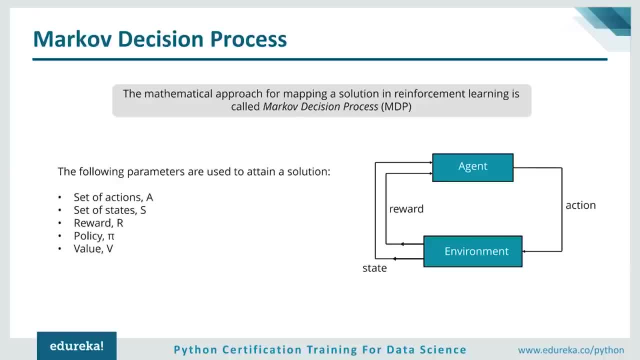 in a way, The purpose of reinforcement learning is to solve a Markov decision process. Okay, So there are a few parameters that are used to get to the solution. So the parameters include the set of actions, the set of states, the rewards, The policy that you're taking to approach the problem and the value that you get. 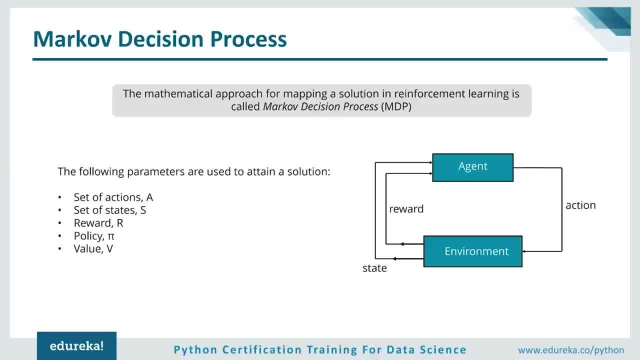 Okay. So to sum it up, the agent must take an action a to transition from a start state to the end state s. while doing so, the agent will receive a reward are for each action that he takes. so, guys, a series of actions taken by the agent define the policy, or it defines the approach and the rewards that are collected. 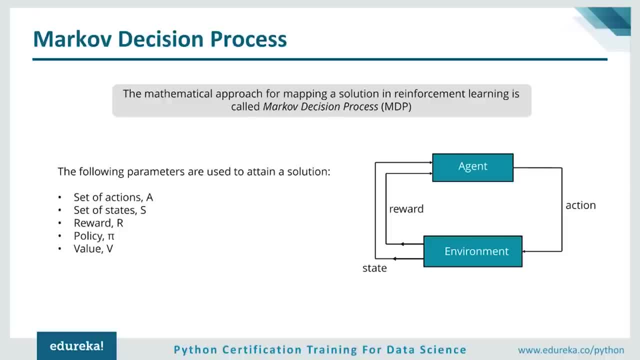 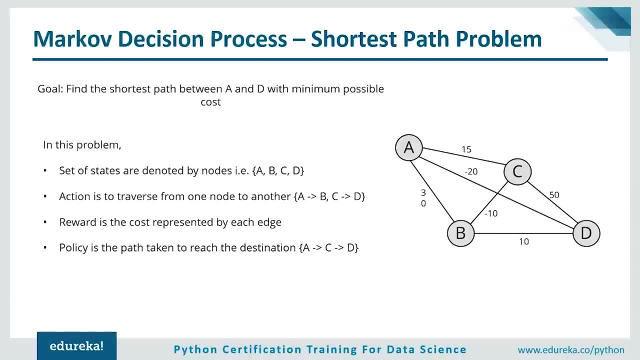 define the value. So the main goal here is to maximize the rewards by choosing the optimum Policy. All right, Now let's try to understand this with the help of the shortest path problem. I'm sure a lot of you might have gone through this problem when you were in college. 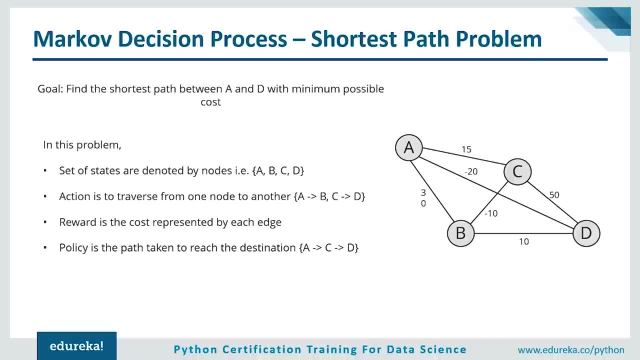 So guys, look at the graph over here. So our aim here is to find the shortest path between A and D with minimum possible cost. So the value that you see on each of these edges basically denotes the cost. So if I want to go from A to C, it's going to cost me 15 points. 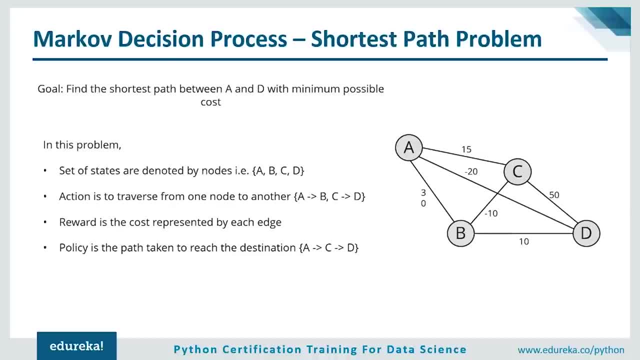 Okay, So let's look at how this is done now, before we move and look at the problem. In this problem, The set of states are denoted by the nodes, which is ABCD, and the action is to traverse from one node to the other. 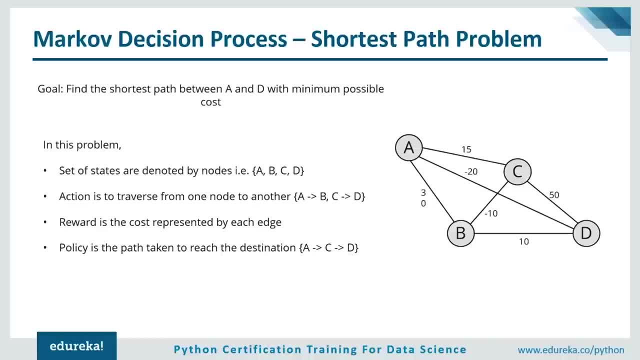 So if I'm going from A to B, that's an action. similarly, A to C, that's an action. Okay, the reward is basically the cost, which is represented by each edge over here. All right Now. the policy is basically the path that I choose to reach the destination. 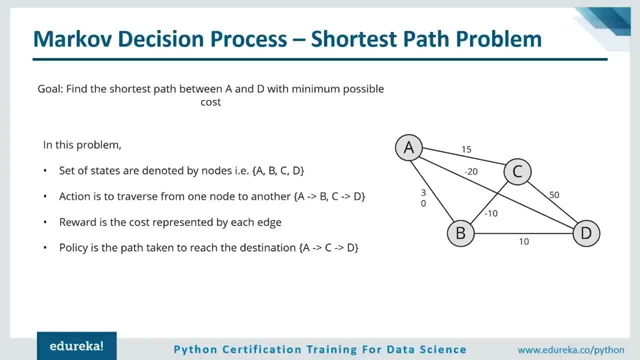 So let's say I choose a CD- Okay, that's one policy. in order to get to D, I'm choosing a CD, which is a policy. Okay, it's basically how I'm approaching the problem. So, guys, here you can start off at node A and you can take baby steps to your destination. 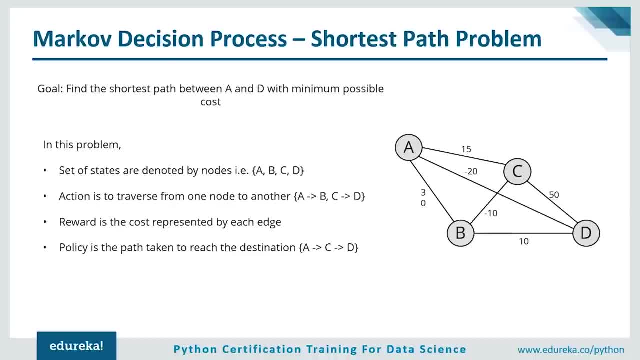 Now, before we move and look at the problem, in this problem, the set of states are denoted by the nodes, which is A, B, C, D, and the action is to traverse from one node to the other. So, if I'm 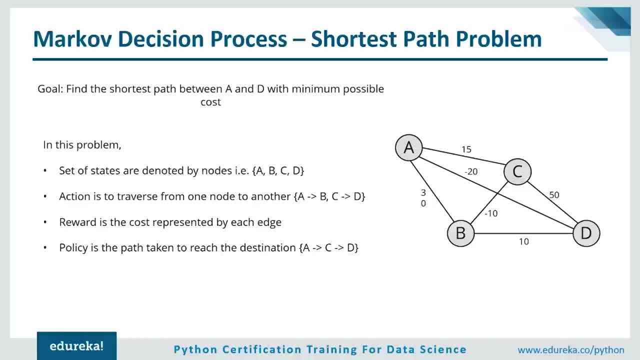 going from A to B. that's an action. Similarly, A to C. that's an action. Okay. The reward is basically the cost which is represented by each edge over here. All right Now. the policy is basically the path that I choose to reach the destination. So let's say I choose A, C, D. Okay, That's one. 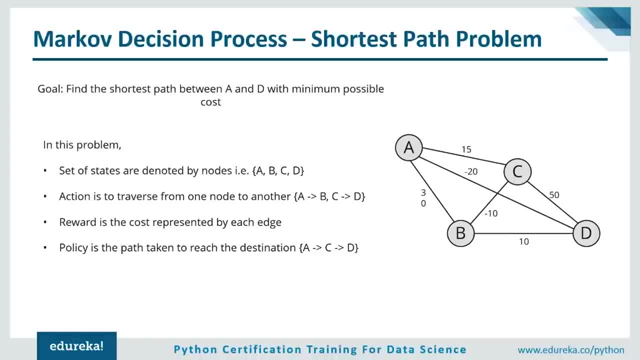 policy In order to get to D, I'm going to choose A C D. So let's say I choose A C D, Which is a policy. Okay, It's basically how I'm approaching the problem. So, guys, here you can. 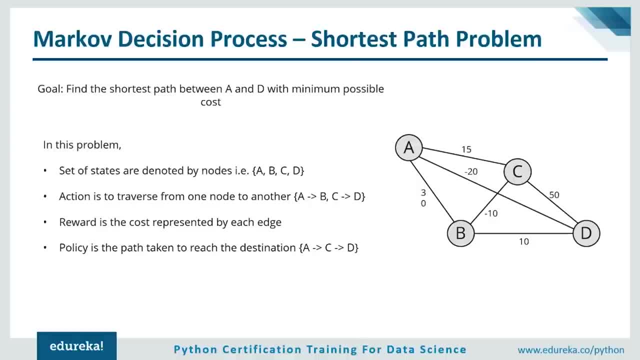 start off at node A and you can take baby steps to your destination Now. initially you're clueless, So you can just take the next possible node which is visible to you. So, guys, if you're smart enough, you're going to choose A to C instead of A B C D or A B D. All right. So now, if you're at node C, 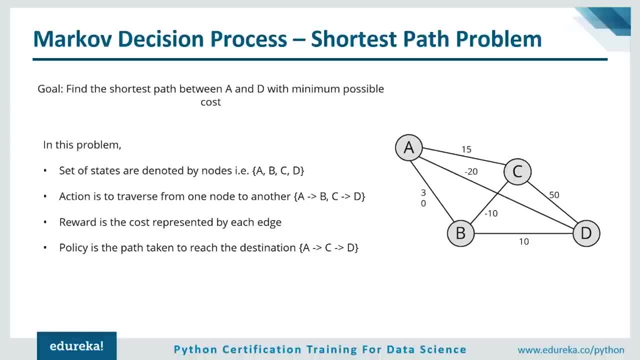 you want to traverse to node D, You must again choose a wise path. All right, You just have to calculate which path you're going to traverse to. So, if you're at node C, you want to traverse to which path has the highest cost or which path will give you the maximum rewards. So, guys, this is a 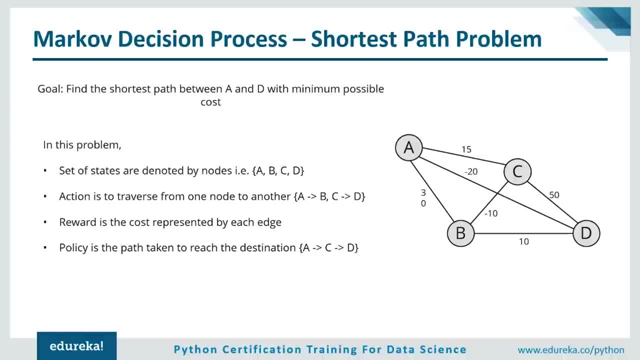 simple problem. We're just trying to calculate the shortest path between A and D by traversing through these nodes. So if I traverse from A, C, D, it gives me the maximum reward. Okay, It gives me 65, which is more than any other policy would give me. Okay. So if I go from A B, D, it would. 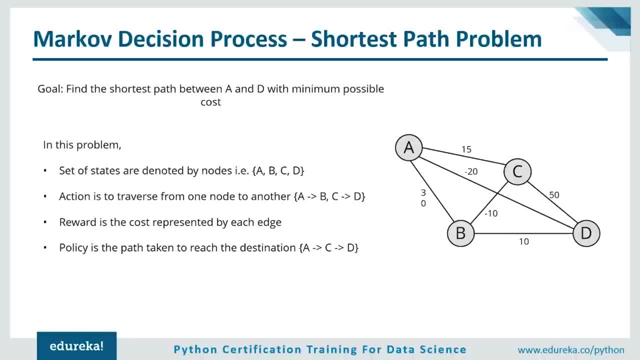 be 40. When you compare this to A C D, it gives me more rewards. So obviously I'm going to go with A C D. Okay, So guys, it was a simple problem. So, guys, if you're at node C, you want to. 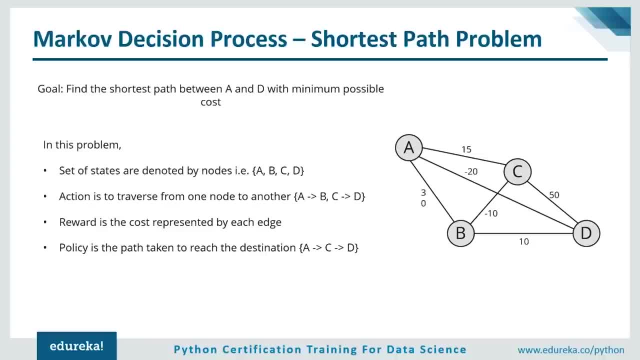 simple problem in order to understand how Markov decision process works. All right, So, guys, I want to ask you a question: What do you think I did here? Did I perform exploration or did I perform exploitation? Now, the policy for the above example is of exploitation, because we didn't explore the 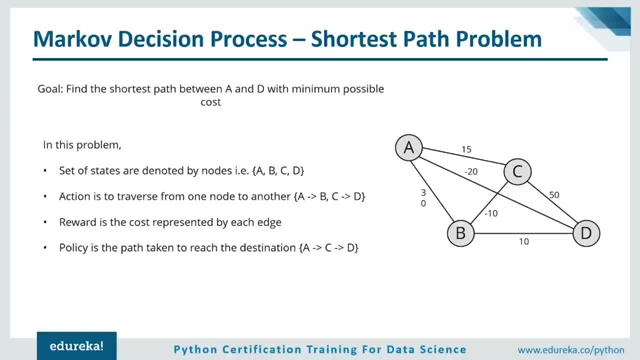 other nodes. Okay, We just selected three nodes and we traverse through them, So that's why this is called exploitation. We must always explore the different nodes so that we can find a more optimal policy, But in this case, obviously, A, C, D has the highest reward. 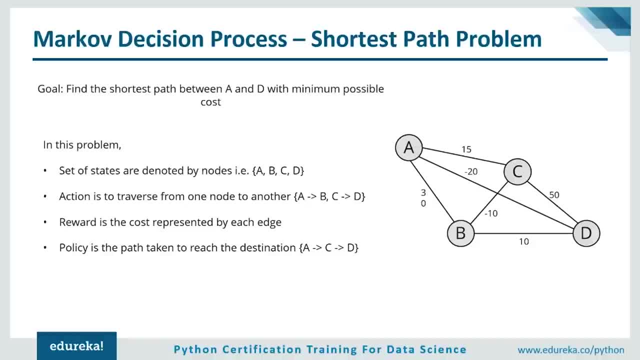 Now, initially you're clueless, So you can just take the next possible node which is visible to you. So guys feel smart enough. You're going to choose A to C instead of ABCD or ABD. All right, So now, if you're at node C, you want to traverse to node D. 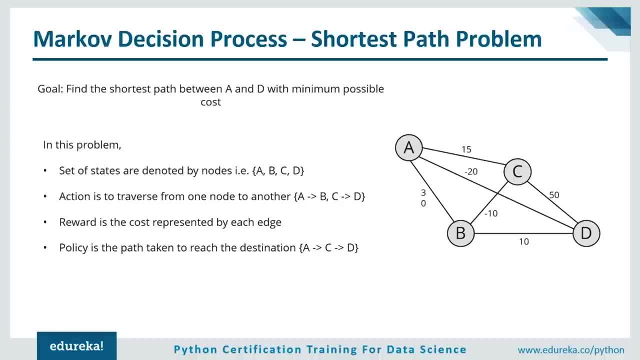 You must again choose a wise path. All right, you just have to calculate which path has the highest cost or which path will give you the maximum rewards. So, guys, this is a simple problem. We're just trying to calculate the shortest path between A and D by traversing through these nodes. 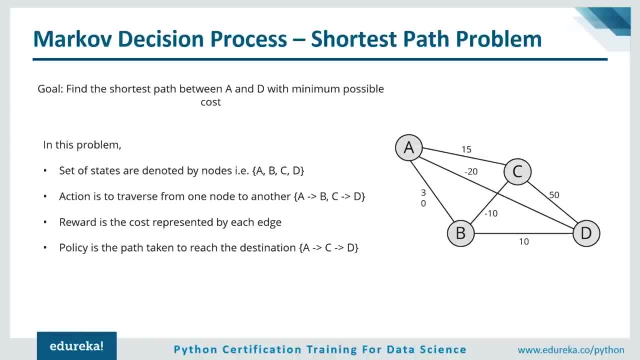 So if I traverse from ACD, it gives me the maximum reward. Okay, it gives me 65, which is more than any other policy would give me. Okay. So if I go from ABD, it would be 40 when you compare this to ACD. 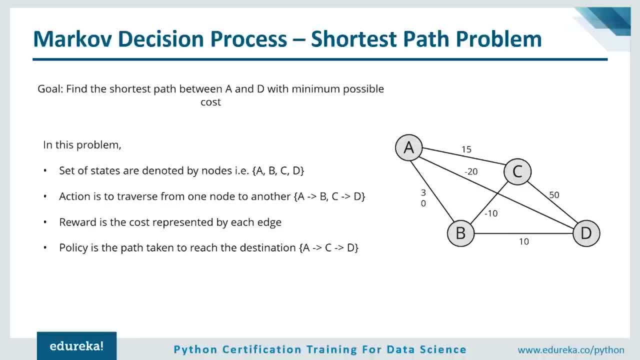 It gives me more rewards, So obviously I'm going to go with ACD. Okay, so, guys, was a simple problem in order to understand how Marco of decision process works, All right. So, guys, I want to ask you a question: What do you think I did here? 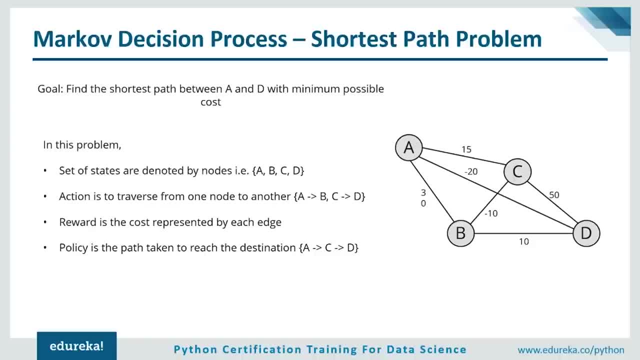 Did I perform exploration or did I perform exploitation? Now, the policy for the above example is of exploitation, because we didn't explore the other nodes. Okay, we just selected three nodes and we traverse through them. So that's why this is called exploitation. 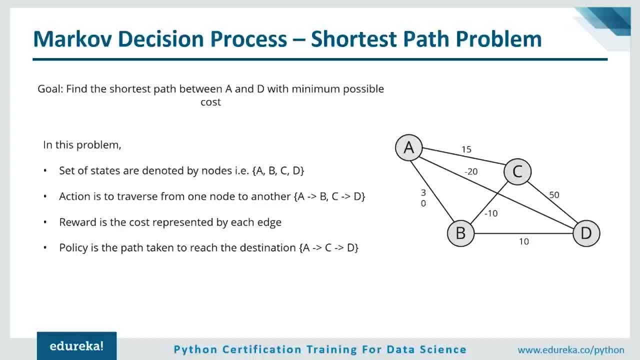 We must always explore the different nodes so that we can find a more optimal policy. But in this case, obviously ACD has the highest reward and we're going with ACD. But generally it's not so simple. There are a lot of nodes. 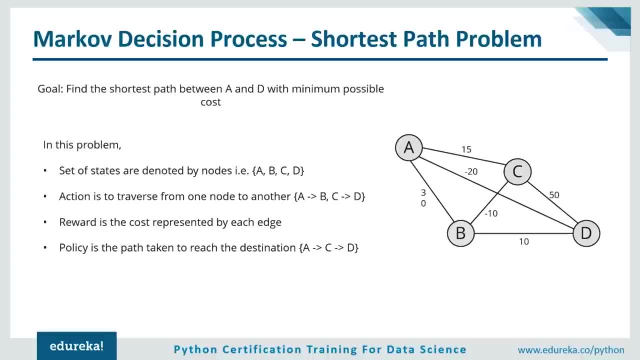 There are hundreds of nodes to Traverse and they're like 50: 60 policies. Okay, 50, 60 different policies. So you make sure you explore through all the policies and then decide on an optimum policy which will give you a maximum reward. 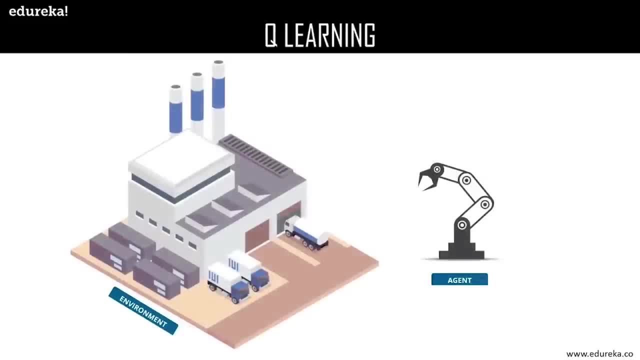 Now for a robot, and environment is a place where it has been put to use. now, Remember, this robot is itself the agent, for example, an automobile factory, where a robot is used to move materials from one place to another. Now, the task we discussed just now have a property in common. 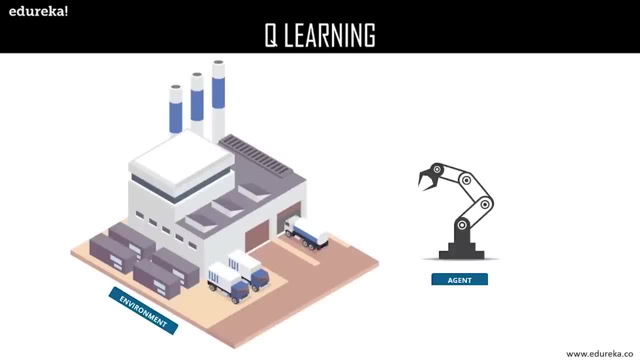 Now, these tasks involve an environment and expect the agent to learn from the environment. Now this is where traditional machine learning fails and hence the need for reinforcement learning. Now it is good to have an established overview of the problem that is to be solved using the Q learning or the reinforcement learning. 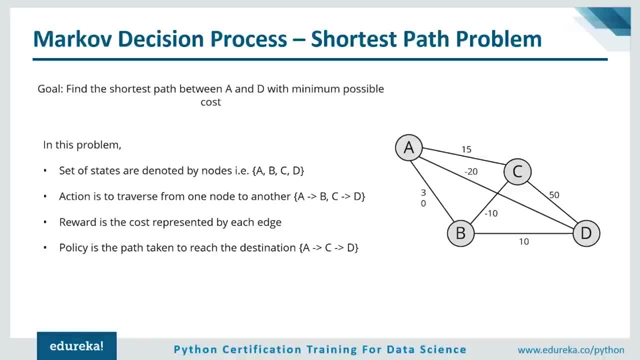 And we're going with A, C, D, but generally it's not so simple. There are a lot of nodes, There are hundreds of nodes to traverse and they're like 50- 60 policies. Okay, 50, 60 different. 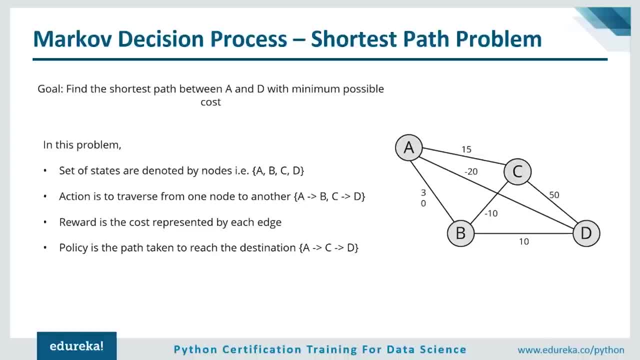 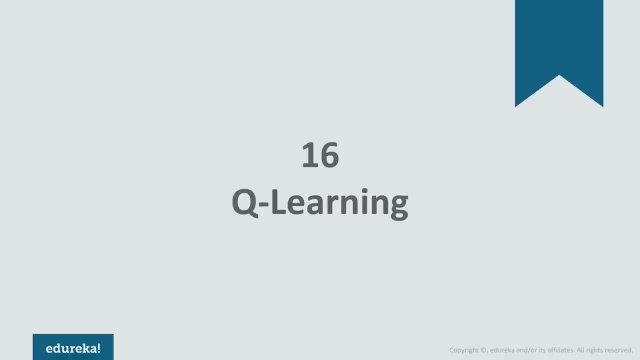 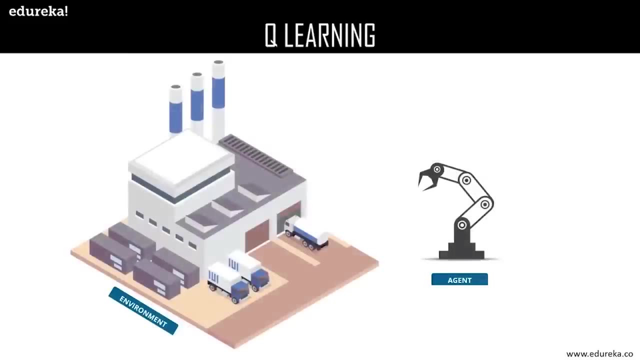 policies. So you make sure you explore through all the policies and then decide on an optimum policy which will give you a maximum reward. Now for a robot, and environment is a place where it has been put to use. Now, remember, this robot is itself the agent. 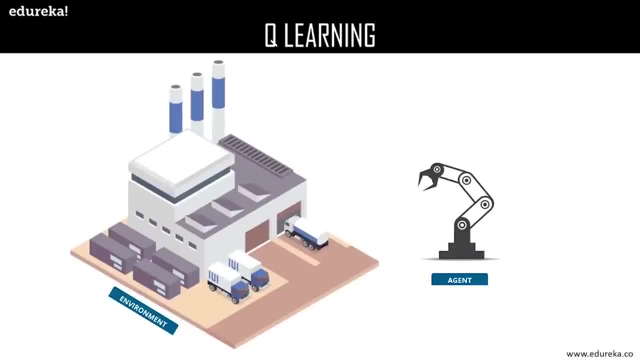 For example, an automobile factory where a robot is used to move materials from one place to another. Now, the task we discussed just now have a property in common. Now, these tasks involve an environment and expect the agent to learn from the environment. Now, this is where traditional machine learning 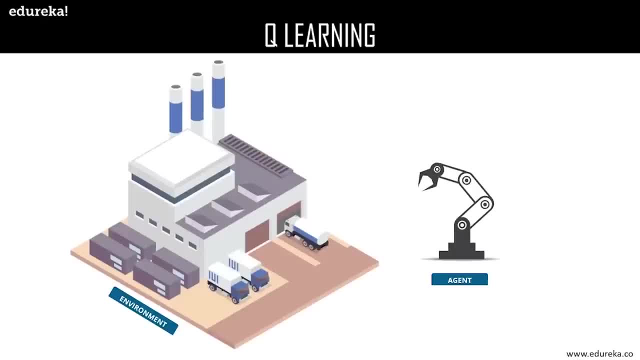 fails, and hence the need for reinforcement learning. Now it is good to have an established overview of the problem that is to be solved using the Q learning or the reinforcement learning. So it helps to define the main components of a reinforcement learning solution, that is, the agent, environment, action, rewards and states. 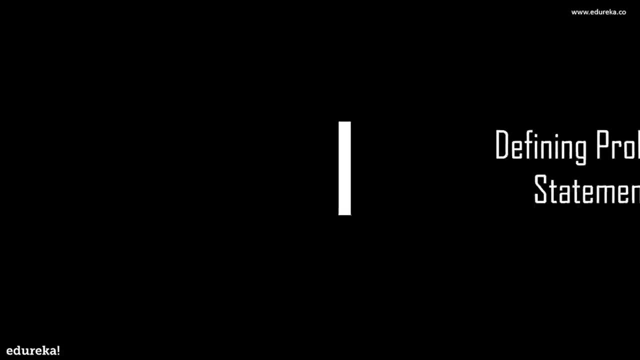 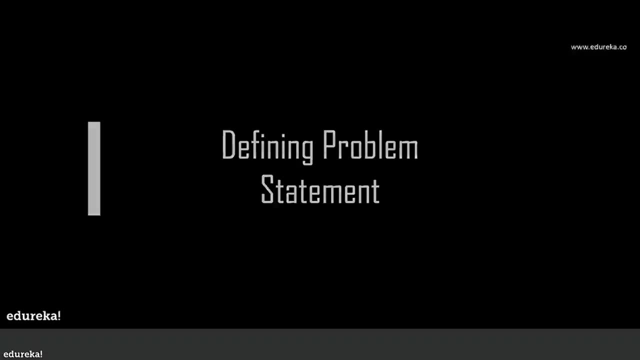 So let's suppose we are to build a few autonomous robots for an automobile building factory. Now These robots will help the factory personal by conveying them the necessary parts that they would need in order to build the car. Now these different parts are located at nine different 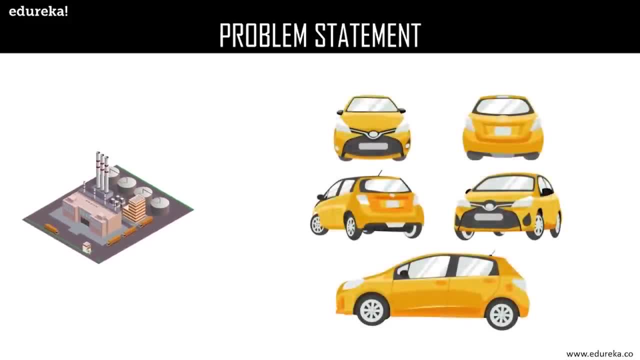 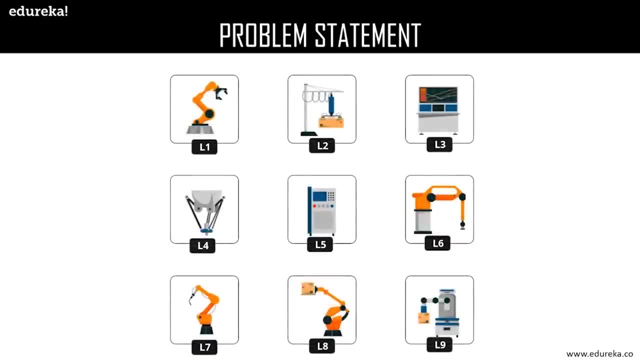 positions within the factory warehouse. the car part include the chassis, wheels, dashboard, the engine and so on, and the factory workers have prioritized the location that contains the body or the chassis to be the topmost, but they have provided the priorities for other locations as well, which? 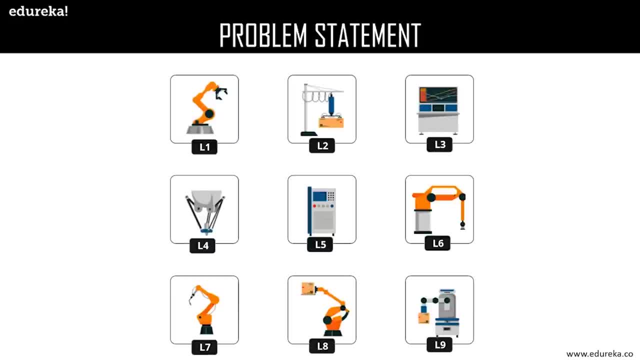 we will look into the moment now. these locations within the factory look somewhat like this. so, as you can see, here we have l1, l2, l3, all of these stations. now one thing you might notice here that there are little obstacle present in between the locations. so l6 is the top priority location. that. 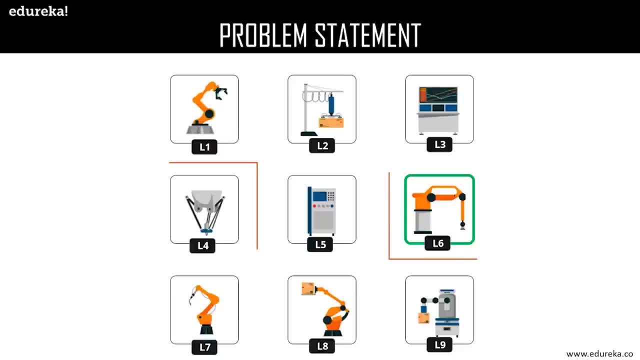 contains the chassis for preparing the car bodies. now the task is to enable the robots so that they can find the shortest route from any given location to another location on their own. now the agents in this case are the robots. the environment is the automobile factory warehouse. so let's talk about 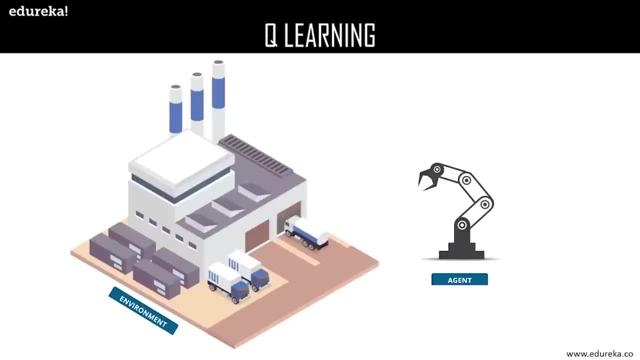 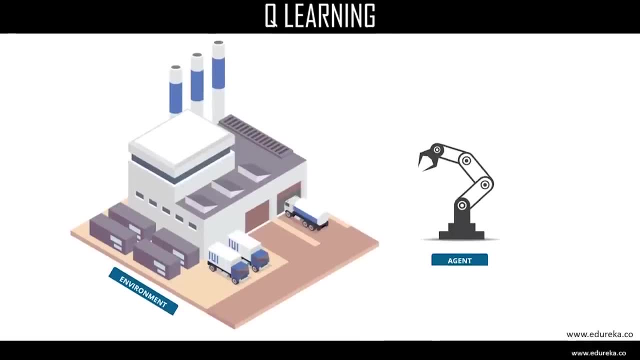 So it helps to define the main components of a reinforcement learning. So it helps to define the main components of a reinforcement learning solution, That is, the agent, environment, action, rewards and States. So let's suppose we are to build a few autonomous robots for an automobile building factory. 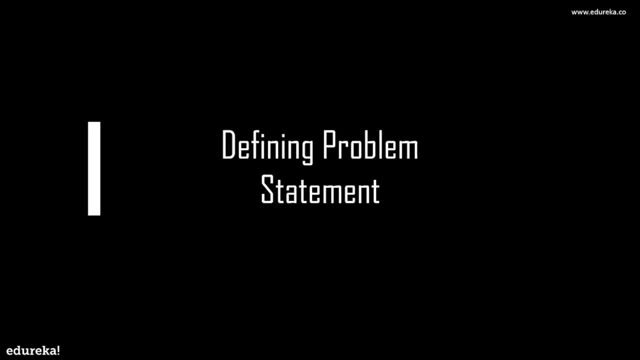 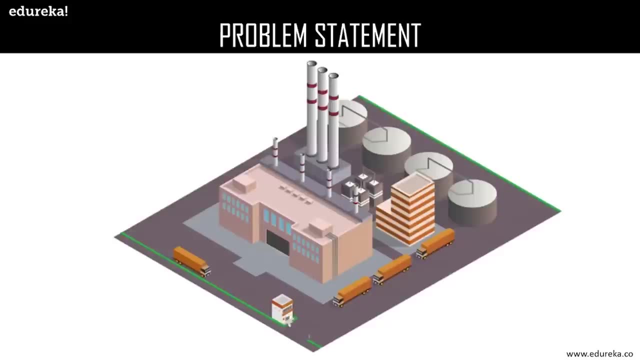 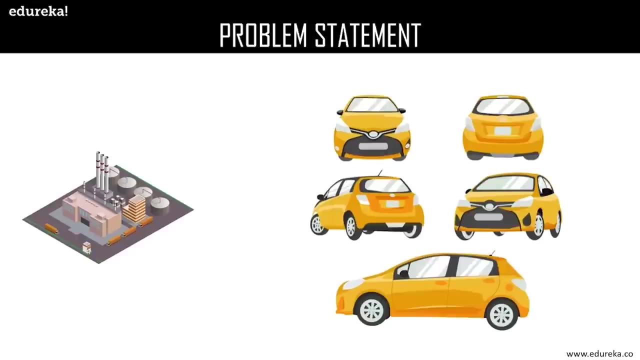 Now these robots will help the factory personal by conveying them the necessary parts that they would need in order to build the car. Now these different parts are located at nine different positions within the factory warehouse. The car part include these: chassis, wheels, dashboard, the engine and so on. 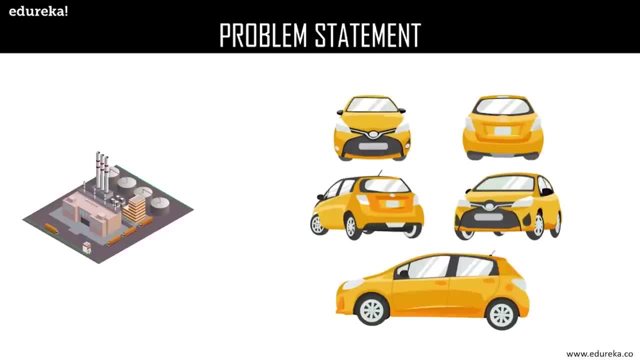 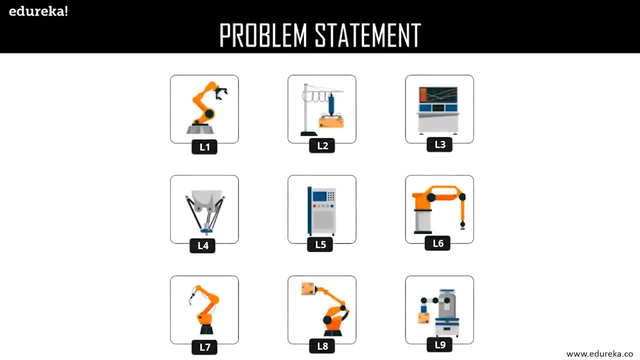 And the factory workers have prioritized the location that contains the body or the chassis to be the topmost, But they have provided the priorities for other locations as well, which we will look into the moment Now. these locations within the factory look somewhat like this: 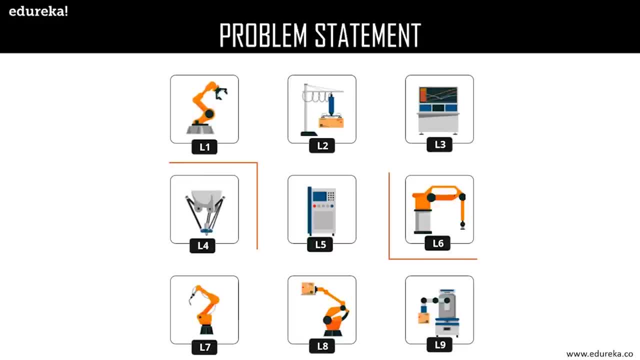 So, as you can see here we have L1, L2, L3, all of these stations. Now, one thing you might notice here that there are little obstacle present in between the locations. So L6 is the top priority Location that contains the chassis for preparing the car bodies. 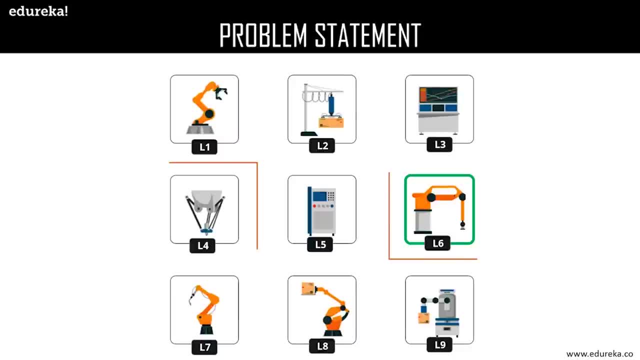 Now the task is to enable the robots so that they can find the shortest route from any given location to another location on their own. Now the agents in this case are the robots. The environment is the automobile factory warehouse. Let's talk about the States. 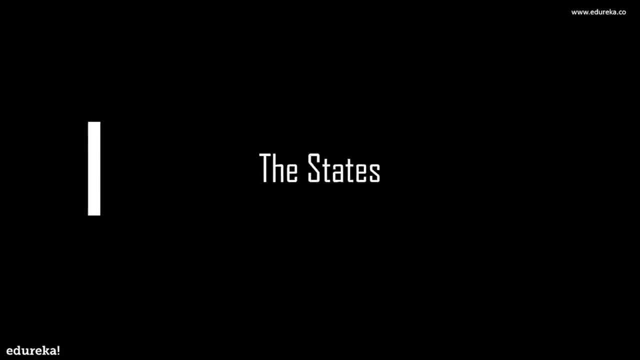 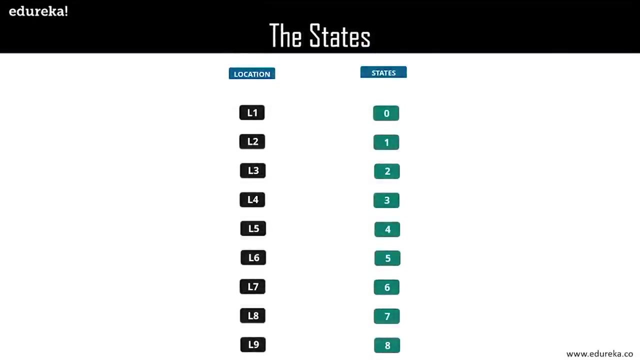 The States are the location in which a particular robot is present in the particular instance of time, which will denote its States. The machines understand numbers Rather than letters, So let's map the location codes to number. So, as you can see here, we have mapped location L1 to the State 0, L2 and 1, and so on. 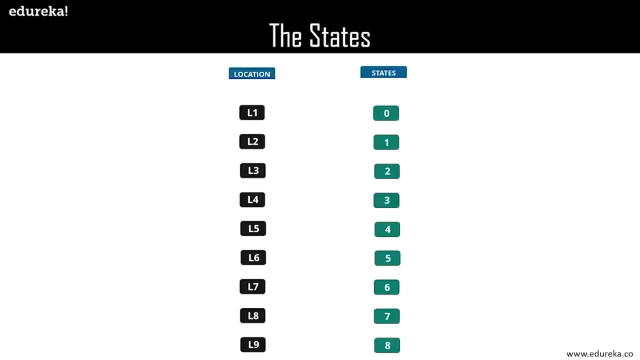 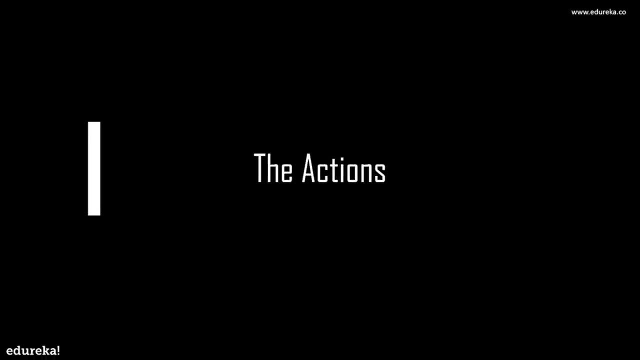 We have L8 as State 7 and N line at State 8.. Well, next, what we're going to talk about are the actions. So in our example, the action will be the direct location that a robot can go from a particular location, right? 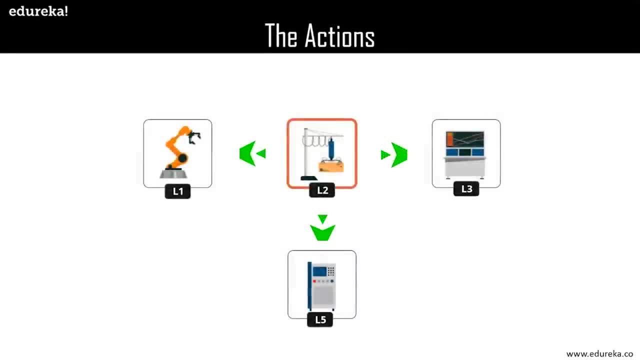 Consider a robot that is at L2 location and the direct locations to which it can move are L5., L1 and L3.. Now the figure here may come in handy to visualize this. Now, as you might have already guessed, the set of actions here is nothing but the set of all possible States of the robot for each location. 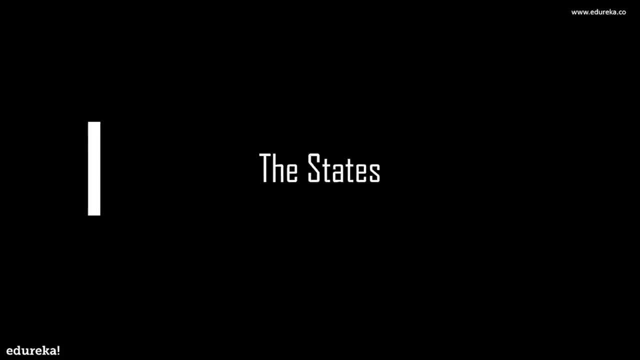 the states. so the states are the location in which a particular robot is located, and the environment is the factory warehouse. so let's talk about the states. so the robot is present in the particular instance of time which will denote its states. now, machines understand numbers rather than letters, so let's map the location codes to number, so as you can. 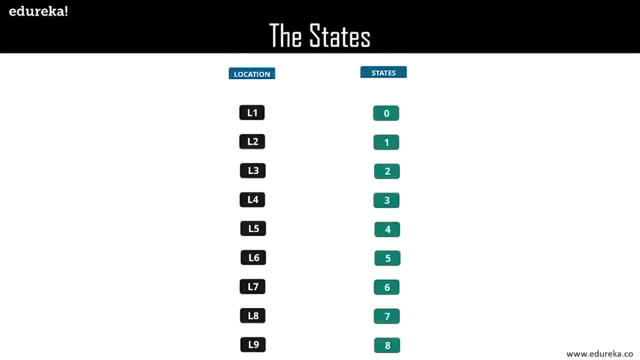 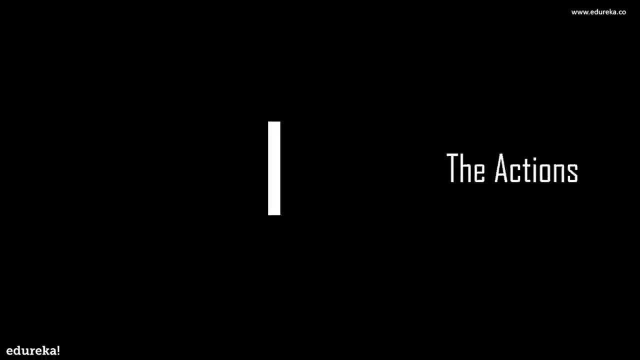 see here we have mapped location l1 to the state 0, l2 and 1 and so on. we have l8 as state 7 and n line at state 8. well, next, what we're going to talk about are the actions. so in our example, the 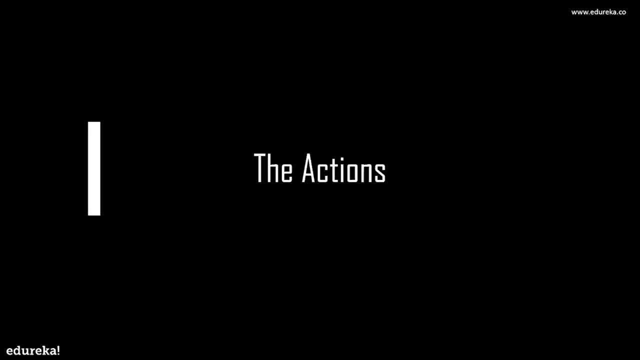 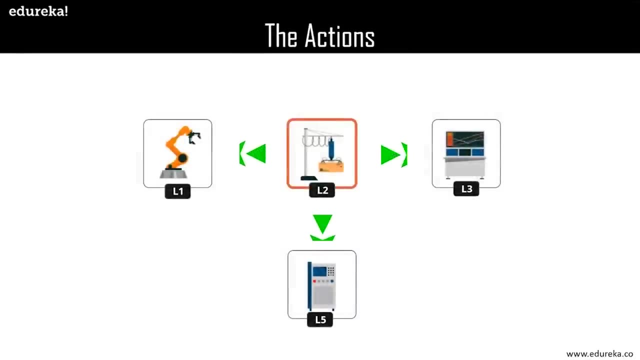 action will be the direct location that a robot can go from a particular location. right, consider a robot that is at l2 location and the direct locations to which it can move are l5, l1 and l3. now, the figure here may come in handy to visualize this now, as you might have already. 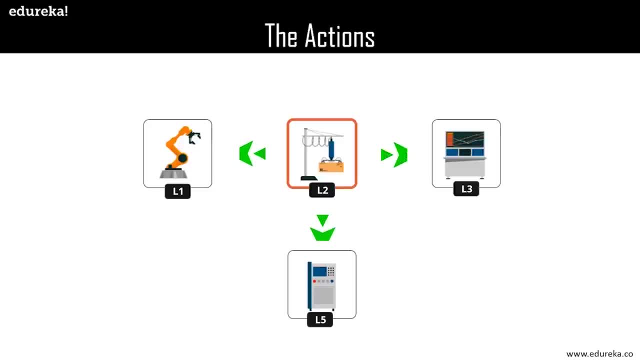 guessed. the set of actions here is nothing but the set of all possible states of the robot. for each location, the set of actions that a robot can take will be different. for example, the set of actions will change if the robot is in l1 rather than l2. all the possible actions will be different. 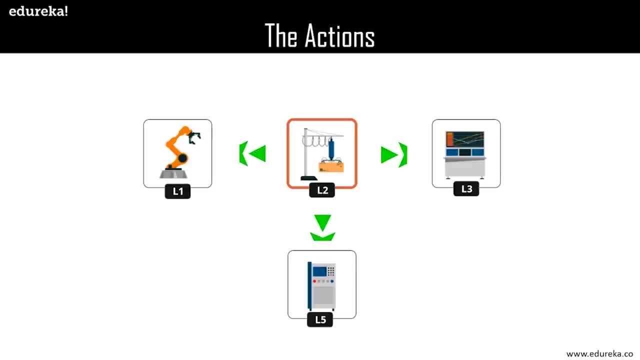 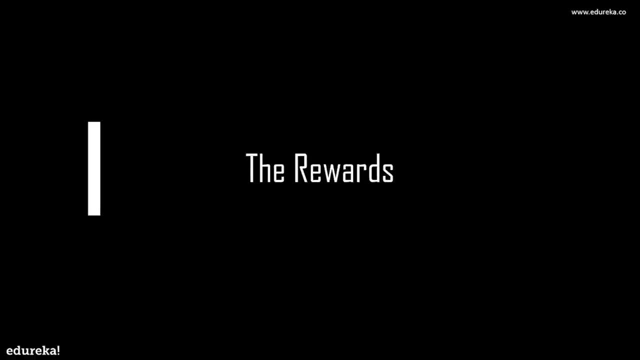 So if the robot is in L1, it can only go to L4 and L2 directly. Now that we are done with the states and the actions, let's talk about the rewards. So the states are basically 0, 1, 2, 3, 4. 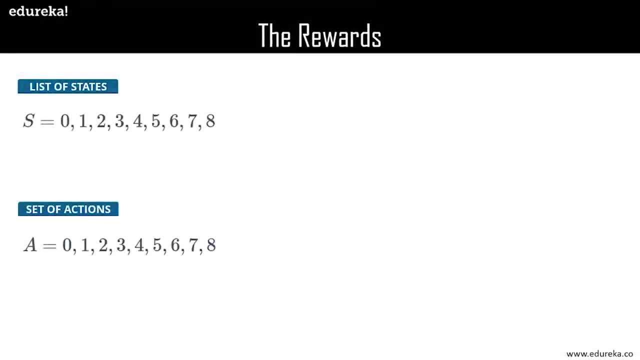 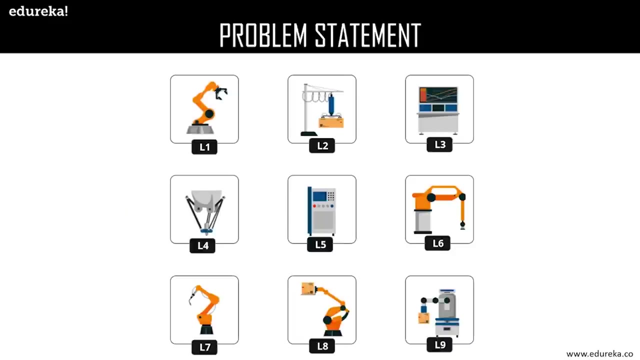 and the actions are also 0, 1, 2, 3, 4, up till 8.. Now the rewards now will be given to a robot if a location, which is the state, is directly reachable from a particular location. So let's take an example: suppose L9 is directly reachable from L8, right? So if a robot goes from L8 to L9 and 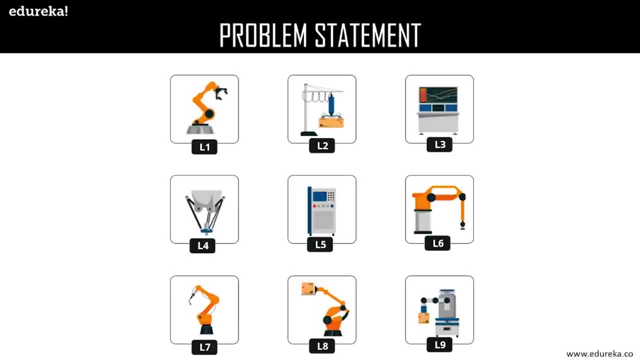 vice versa, it will be rewarded by 1, and if a location is not directly reachable from a particular location, we do not give any reward. a reward of 0.. Now, the reward is just a number here and nothing else. It enables the robots to make sense of the movements, helping them in deciding what locations. 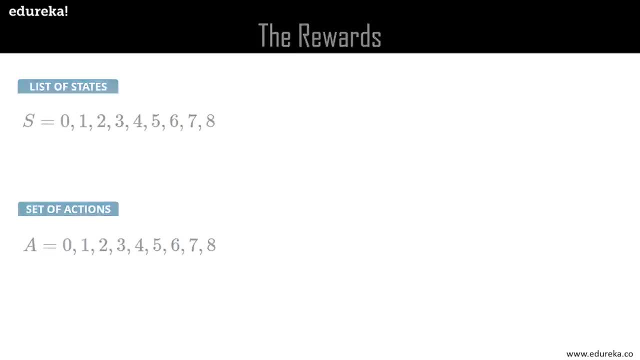 are directly reachable and what are not? Now, with this queue, we can construct a reward table which contains the actions of the state and the actions of the robot. So let's take a look at the reward table, which contains all the reward values, mapping between all possible states. So, as you 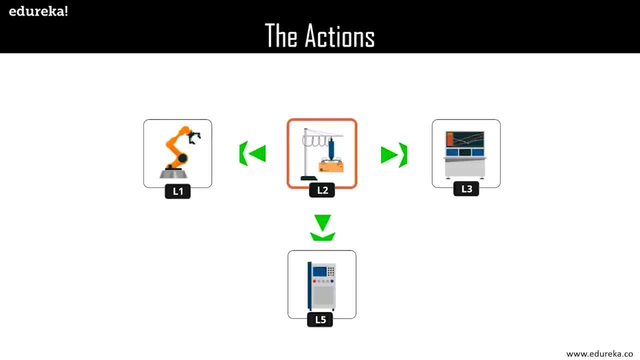 The set of actions that a robot can take will be different. For example, the set of actions will change if the robot is in L1 rather than L2.. So if the robot is in L1, it can only go to L4 and L2 directly. 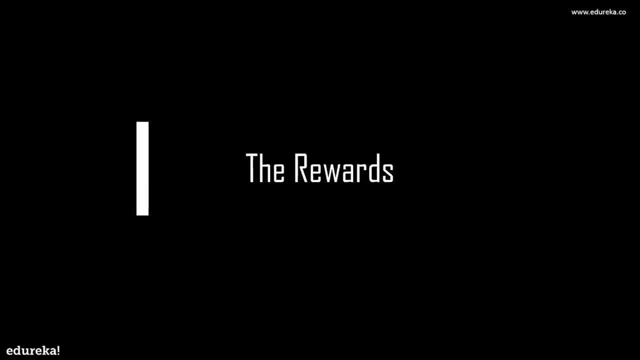 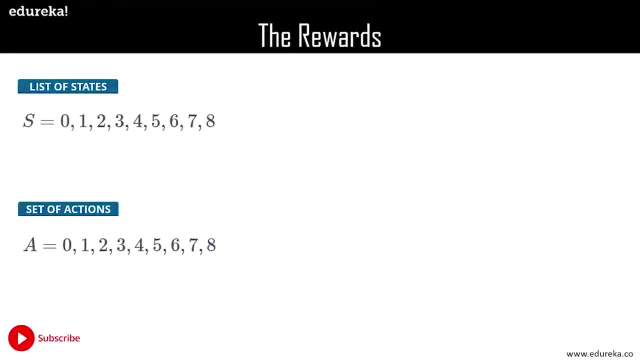 Now that we are done with the states and the actions, let's talk about the rewards. So the states are basically 0, 1, 2, 3, 4, and the actions are also 0, 1, 2, 3, 4 up till 8.. 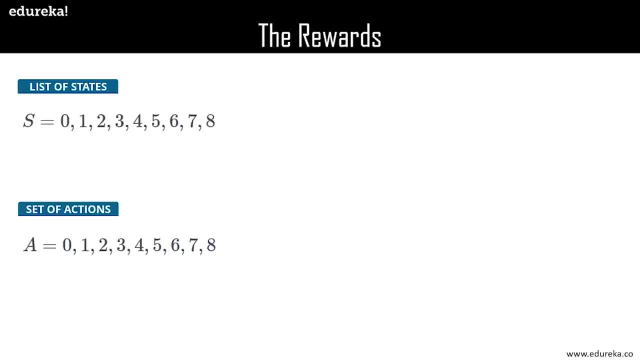 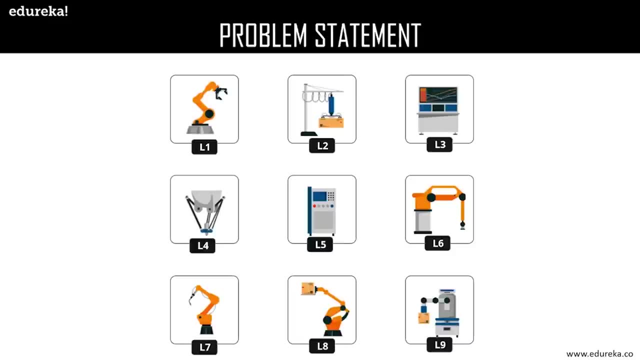 Now the rewards now will be given to a robot if a location, which is the State, is directly reachable from a particular location. So let's take an example: Suppose L9 is directly reachable from L8, right. So if a robot goes from L8 to L9 and vice versa, 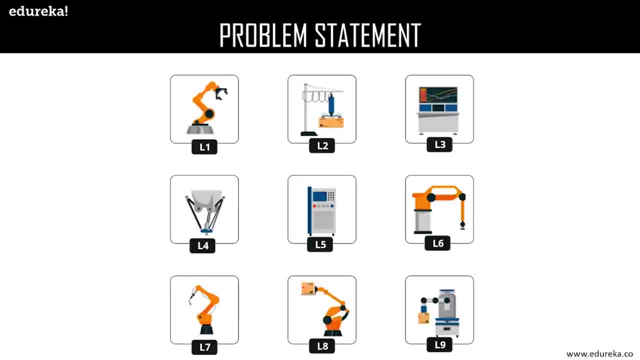 it will be rewarded by one, and if a location is not directly reachable from a particular location, we do not give any reward, a reward of zero. now, the reward is just a number here and nothing else. it enables the robots to make sense of the movements, helping them in deciding what locations. 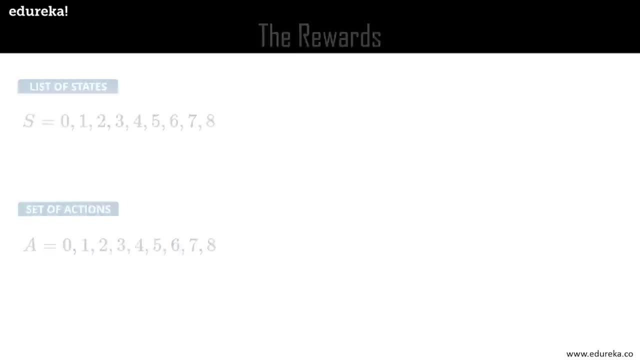 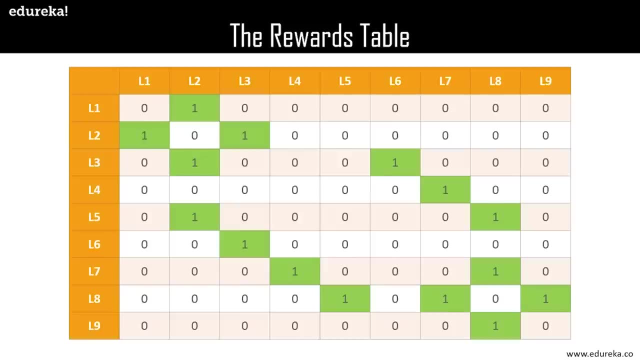 are directly reachable and what are not. now, with this queue, we can construct a reward table which contains all the reward values, mapping between all possible states. so, as you can see here in the table, the positions which are marked green have a positive reward and, as you can see here, 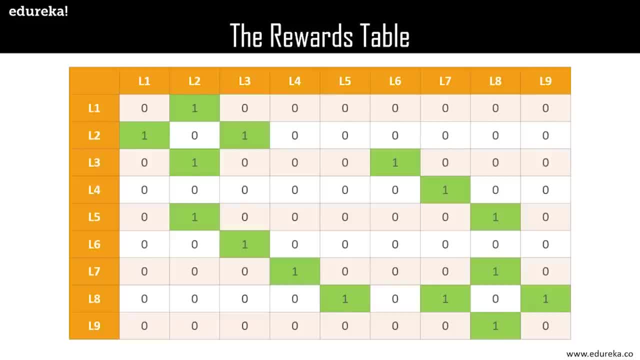 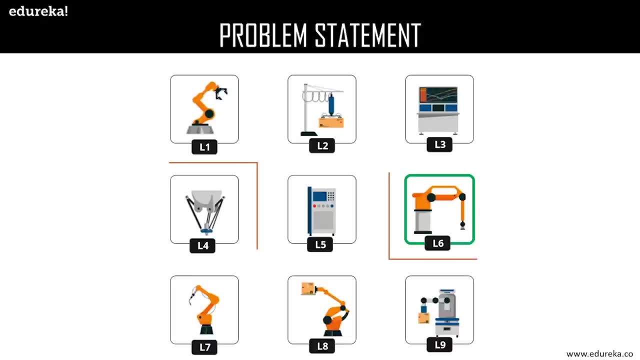 we have all the possible rewards that a robot can get by moving in between the different states. now comes an interesting decision. now remember that the factory administrator prioritized l6 to be the top most. so how do we incorporate this fact in the above table? now this is done. 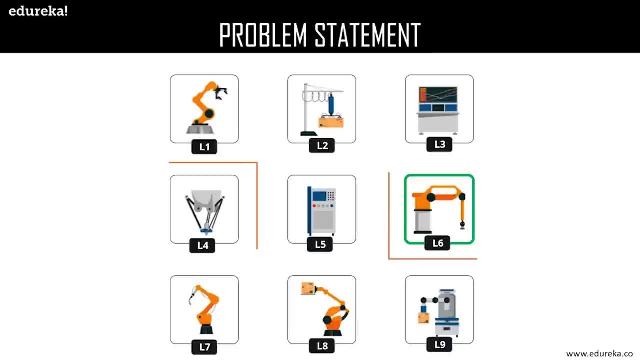 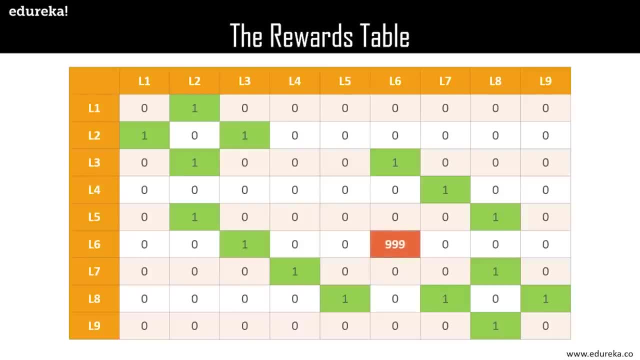 by associating the topmost priority location with a very high reward than the usual ones. so let's put 999 in this table, cell l6, comma l6. now the table of rewards with the higher reward for the top most location looks something like this: we have now formally defined all the vital components for the solution we are 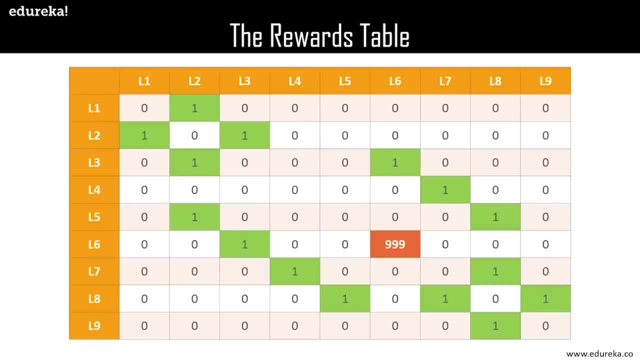 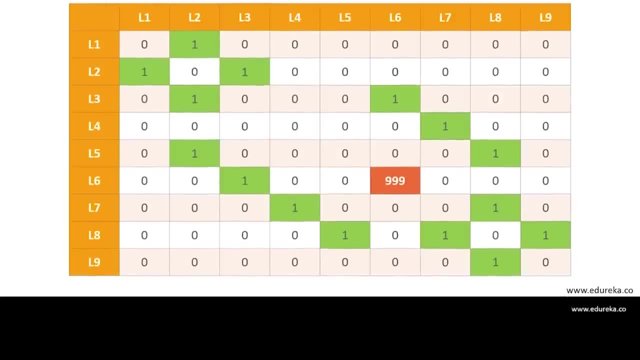 aiming for the problem discussed now, we will shift gears a bit and study some of the fundamental concepts that prevail in the world of reinforcement learning and queue learning. so first of all we'll start with the bellman equation. now consider the following square of rooms, which is analogous to: 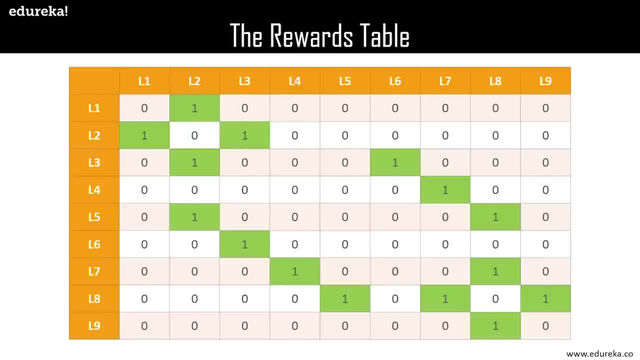 can see here in the table, the positions which are marked green have a positive reward and, as you can see, here we have all the possible rewards that a robot can get by moving in between the different states. Now comes an interesting decision. Now remember that the factory administrator prioritized. 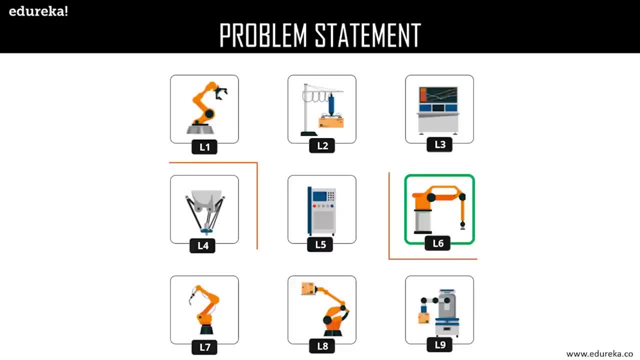 L6 to be the top most. So how do we incorporate this fact in the above table? Now, this is done by associating the top most priority location with the state. So let's take a look at the table with the very high reward than the usual ones. So let's put 999 in the cell L6, L6.. Now the 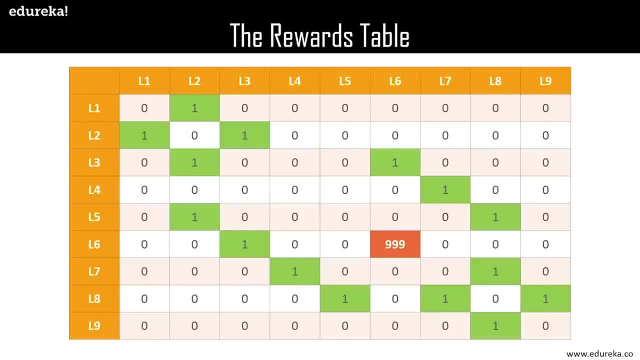 table of rewards, with the higher reward for the top most location, looks something like this: We have now formally defined all the vital components for the solution we are aiming for, the problem discussed now. We will shift gears a bit and study some of the fundamental concepts that prevail in 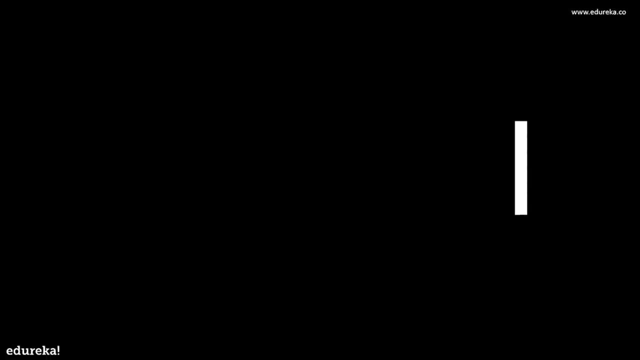 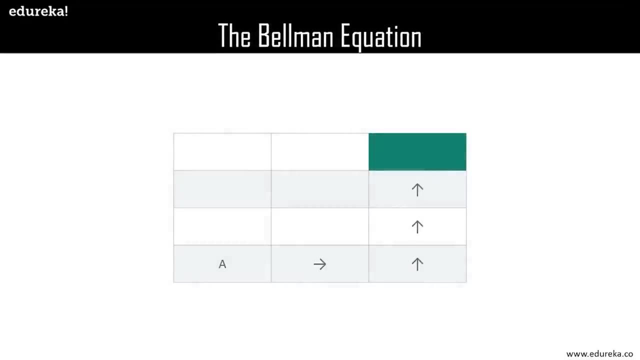 the world of reinforcement learning and queue learning. So first of all we'll start with the Bellman equation. Now consider the following square of rooms, which is analogous to the actual environment from our original problem, but without the barriers. Now suppose a robot needs to go to. 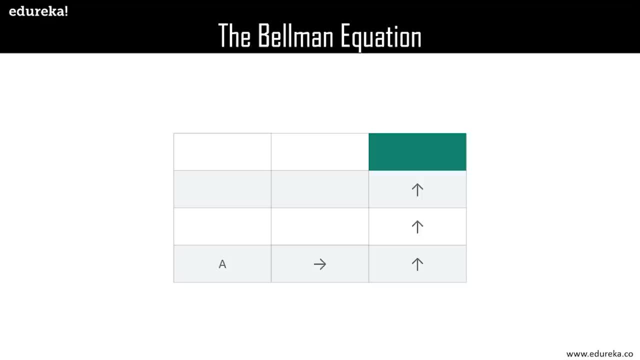 the room marked in the green from its current position A using the specified direction. Now, how can we enable the robot to do this programmatically? One idea would be introduce some kind of a footprint which the robot will be able to follow. Now, here a constant value is specified in each of the rooms which will come along the robot's. 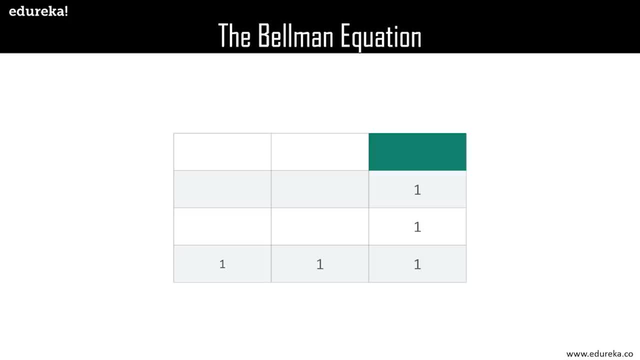 way if it follows the direction specified above now. in this way, if it starts at location a, it will be able to scan through this constant value and will move accordingly. but this will only work if the direction is prefixed and the robot always starts at the location a. now consider the robot. 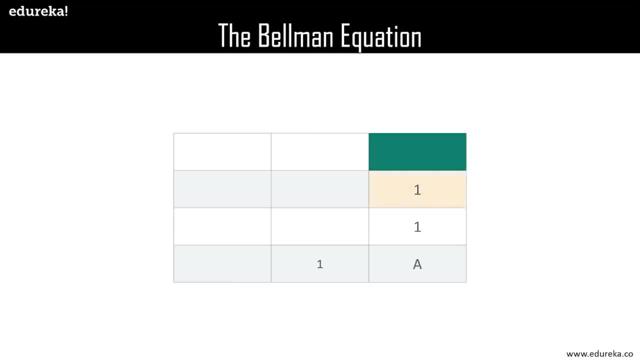 starts at this location rather than its previous one. now, the robot now sees footprints in two different directions. it is therefore unable to decide which way to go in order to get the destination, which is the green room. it happens primarily because the robot does not have a way. 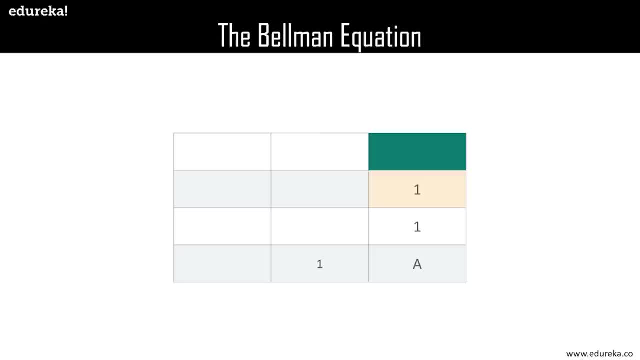 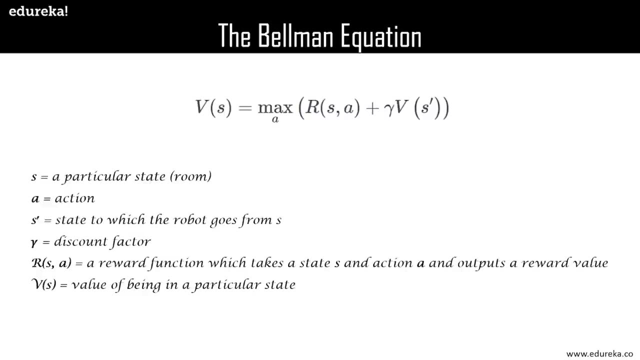 to remember the directions to proceed. so our job now is to enable the robot with a memory. now, this is where the bellman equation comes into play. so, as you can see here, the main reason of the bellman equation is to enable the robot with the memory. that's the thing we're going to use. 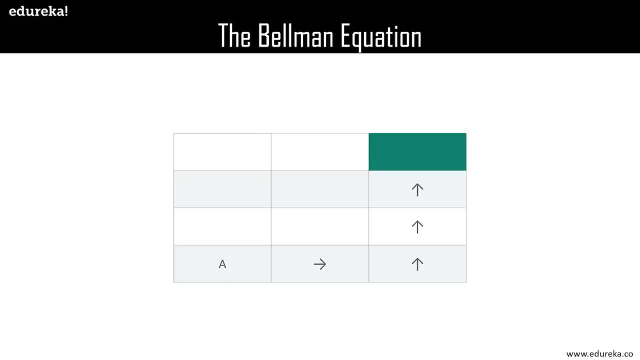 the actual environment from our original problem, but without the barriers. now suppose a robot needs to go to the room marked in the green from its current position, a, using the specified direction. now, how can we enable the robot to do this programmatically? one idea would be introduced, some kind of a footprint which the robot will be able 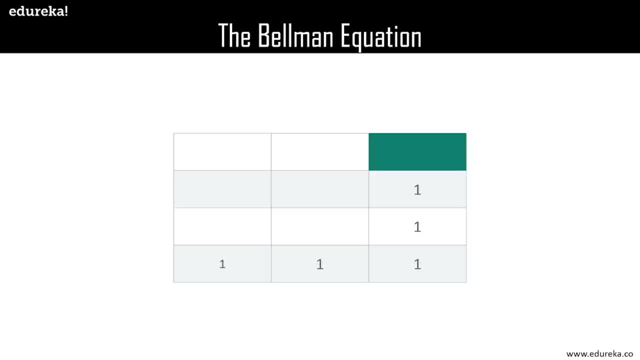 to follow. now here a constant value is specified in each of the rooms which will come along the robots way if it follows the direction specified above now. in this way, if it starts at location a, it will be able to scan through this constant value and will move accordingly. but this will only work if the direction 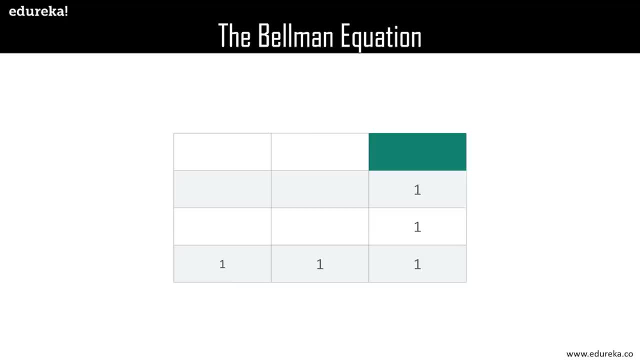 is prefixed and the robot always starts at the location a. now consider: the robot starts at this location rather than its previous one. now, the robot now sees footprints in two different directions. it is therefore unable to decide which way to go in order to get the destination, which is the green room. it. 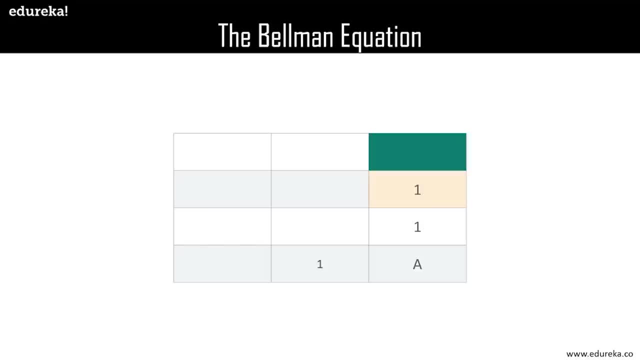 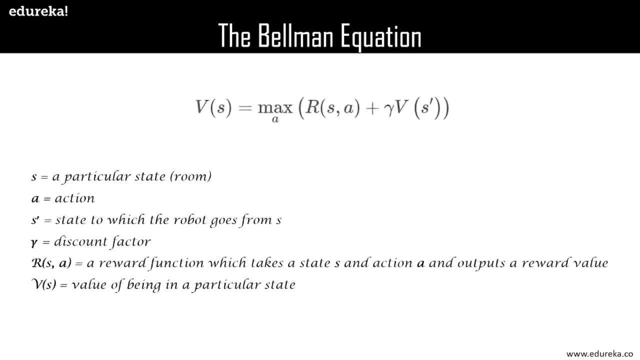 happens primarily because the robot is unable to decide which way to go in order to get the destination, which is the green room. it happens primarily because the robot does not have a way to remember the directions to proceed. so our job now is to enable the robot with the memory. now, this is where the Bellman 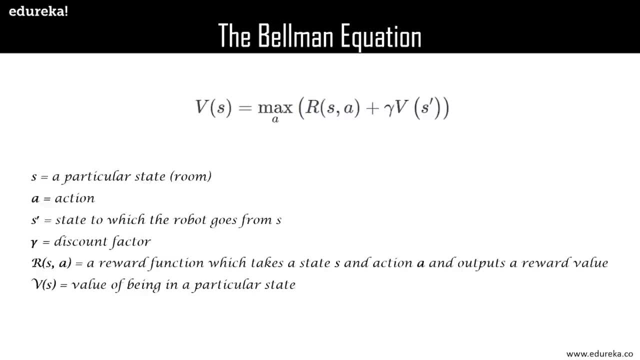 equation comes into play. so, as you can see here, the main reason of the Bellman equation is to enable the robot with the memory- that's the thing we're going to use. so the equation goes something like this: V of s gives maximum of a R of s. 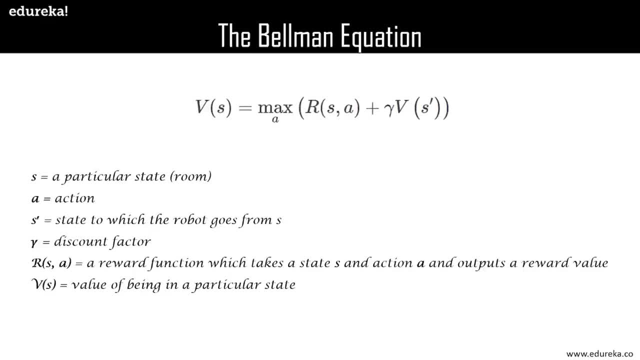 comma a plus gamma of V, s- where s is a particular state, which is the room, a is the action moving between the rooms s dash is the state to which the robot goes from. s and gamma is the discount factor- now we'll get into it in a moment- and obviously, r of s comma a. 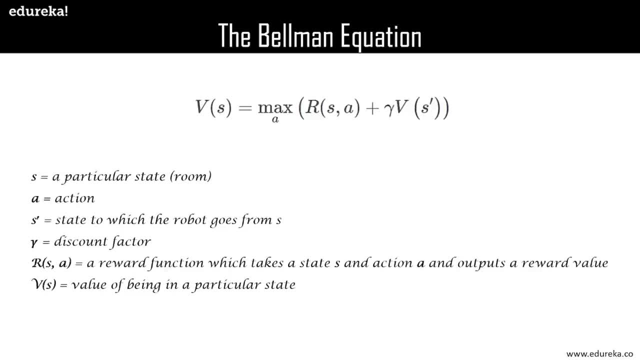 is a reward function which takes a state s and action a and outputs the reward. now, v of s is the value of being in a particular state, which is the footprint. now we consider all the possible actions and take the one that yields the maximum value. now there is one constraint, however, regarding 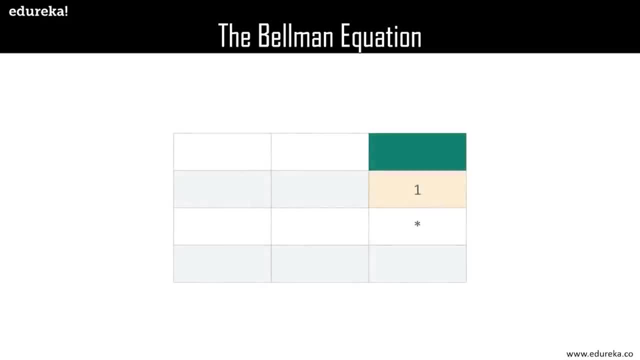 the value footprint. that is the room marked in the yellow just below the green room. it will always have the value of one to denote that is one of the nearest room, adjacent to the green room. now, this is also to ensure that a robot gets a reward when it goes from a yellow room to the green room. 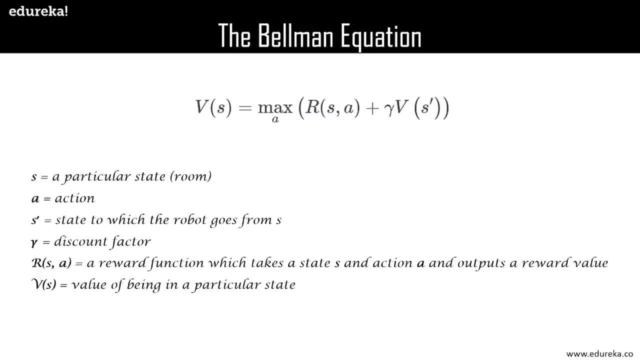 so the equation goes something like this: v of s gives maximum of a r of s comma a, plus gamma of v of s comma a. so v of s becomes small investigations. the r of s good ا is male. then we can see that y gives us value of. z is the line of error for two functions. so we can think: 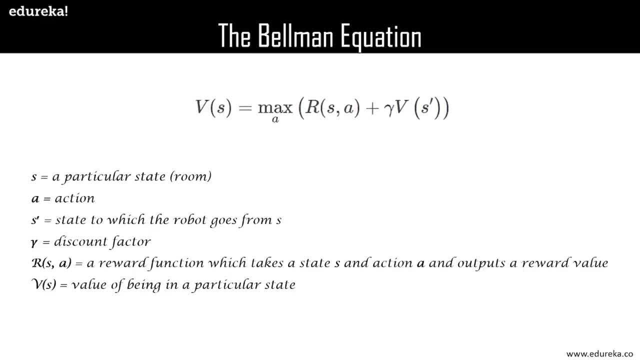 where s is a particular state which is a room. a is the action moving between the rooms s, dash is the state to which the robot goes from. s and gamma is the discount factor- now we'll get into it in a moment- and obviously r of s comma a is a reward function which takes a state s. 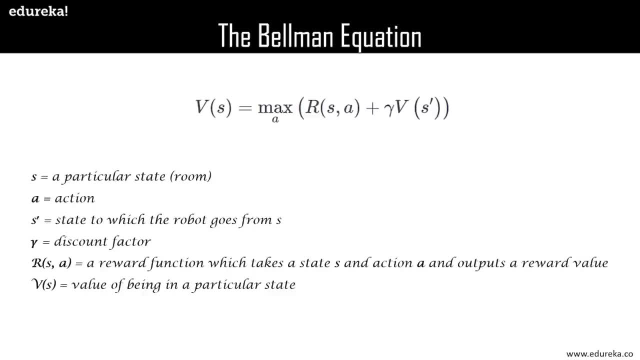 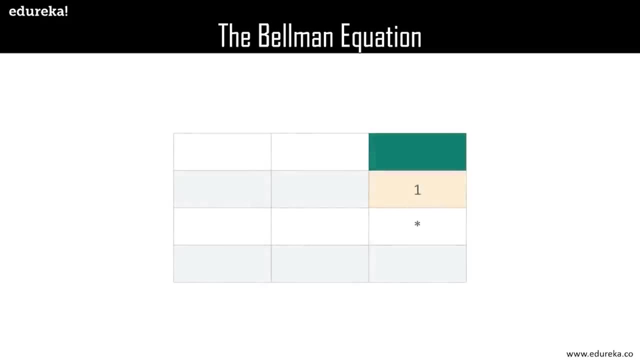 and action a and outputs. the reward now, v of s, is the value of being in a particular state, which is the footprint. now we consider all the possible actions and take the one that yields the maximum value. now there is one constraint, however, regarding the value footprint, that is, the room marked in the 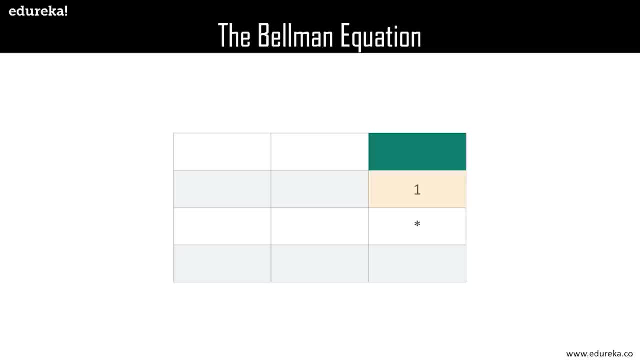 yellow just below the green room, it will always have the value of one to denote that is one of the nearest room, adjacent to the green room. now, this is also to ensure that a robot gets a reward when it goes from a yellow room to the green room. let's see how to make sense of the equation, which. 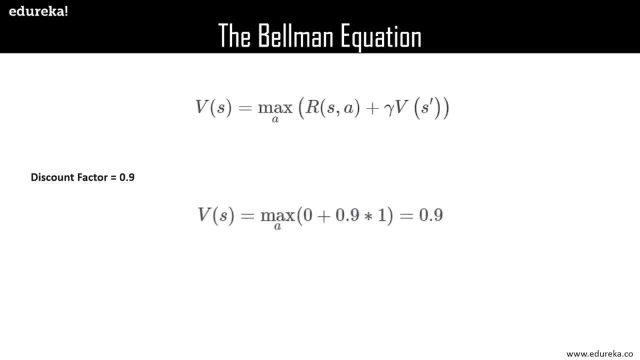 we have here. so let's assume a discount factor of 0.9. as we remember, gamma is the discount value or the discount factor. so let's take it 0.9 now for the room which is marked just below the one, or the yellow room, which is the asterisk mark for this room. what will be the v of s, that is, the value of? 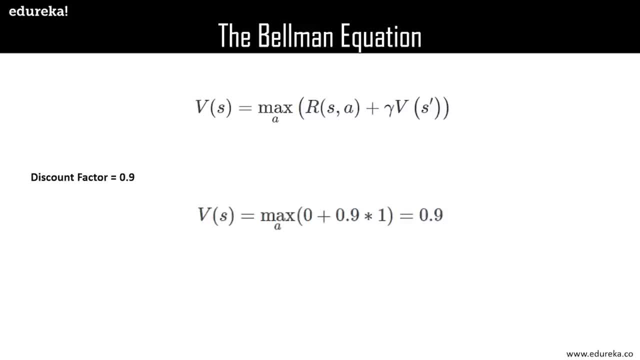 being in a particular state. so for this v of s would be something like: maximum of a will take 0, which is the initial of r s comma a, plus 0.9, which is gamma, into one that gives us 0.9. now here the robot will not get any reward for going to a. 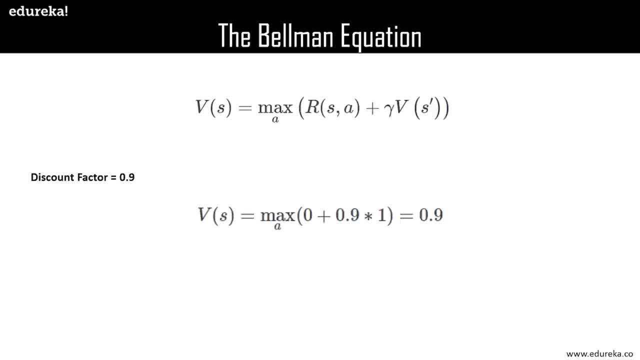 state marked in yellow. hence the rs comma a is 0 here, but the robot knows the value of being in the yellow room, hence v of s dash is one. following this for the other states, we should get 0.9. then again, if we put 0.9 in this ecuation, we get 0.81. the zero point seven, two native zero point nine. 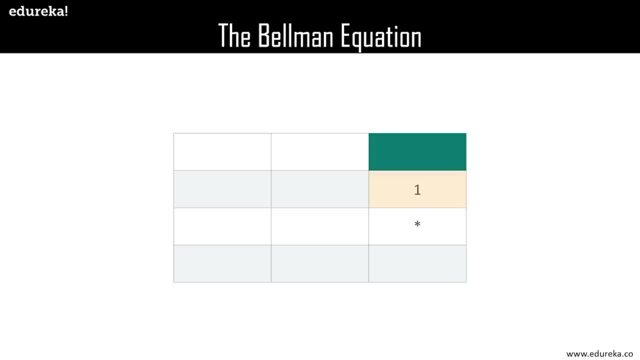 let's see how to make sense of the equation which we have here. so let's assume a discount factor of 0.1, 9. as we remember, gamma is the discount value or the discount factor. so let's take it 0.9 now for. 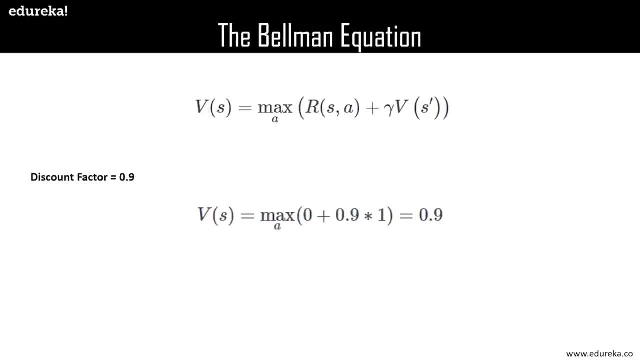 the room which is marked just below the one, or the yellow room, which is the asterisk mark for this room. what will be the v of s? that is, the value of being in a particular state. so for this v of s would be something like: maximum of a will take 0, which is the initial of r s comma a, plus 0.9, which. 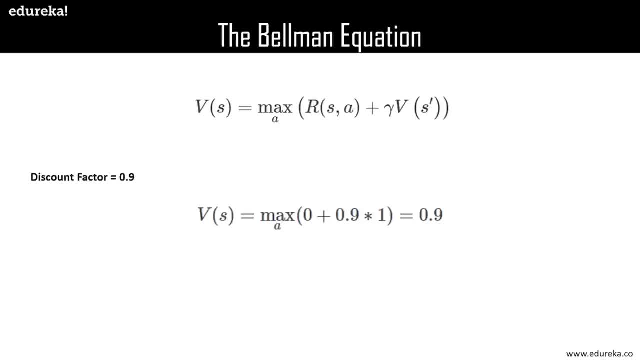 is gamma into 1, that gives us 0.9. now, here the robot will not get any reward for going to a state marked in yellow, hence the r s comma a is 0 here. but the robot knows the value of being in the yellow room, hence v of s dash is 1. 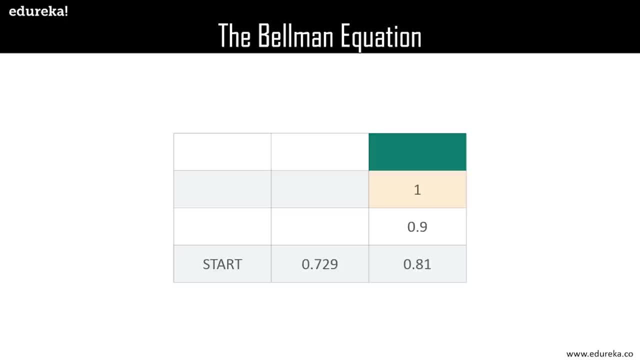 following this for the other states, we should get 0.9. then again, if we put 0.9 in this equation, we get 0.81, then 0.729 and then we again reach the starting point. so this is how the table looks, with some value footprints computed from the bellman equation. 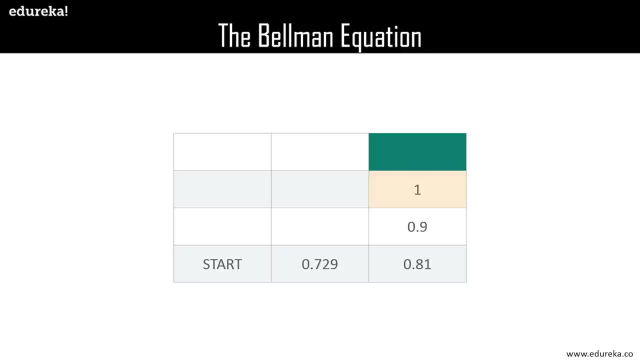 now, a couple of things to notice here is that the max function helps the robot to always choose the state that gives it the maximum value of being in that state. now the discount factor, gamma, notifies the robot about how far it is from the destination. this is typically specified by the developer of 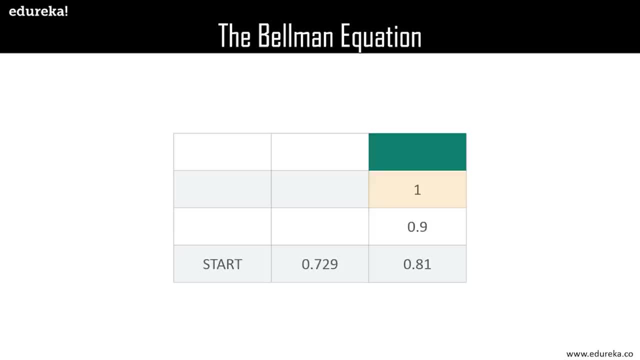 the algorithm that would be installed in the robot. now the other states can also be given their respective values. so this is how the table looks, with some value footprints computed from the bellman equation values. in a similar way, so, as you can see here, the boxes adjacent to the green one have one. 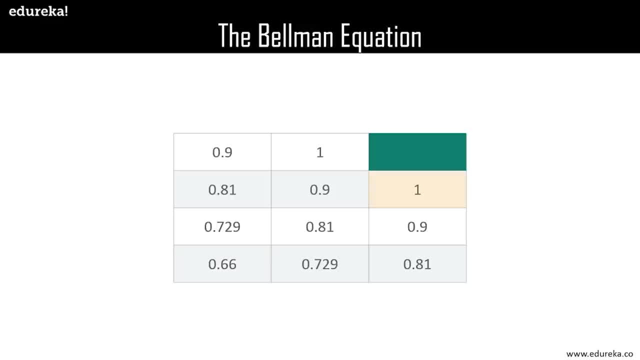 and if we move away from one, we get 0.9, 0.81, 0.729 and finally we reach 0.66. now the robot now can proceed its way through the green room utilizing these value footprints, even if it's dropped at any. 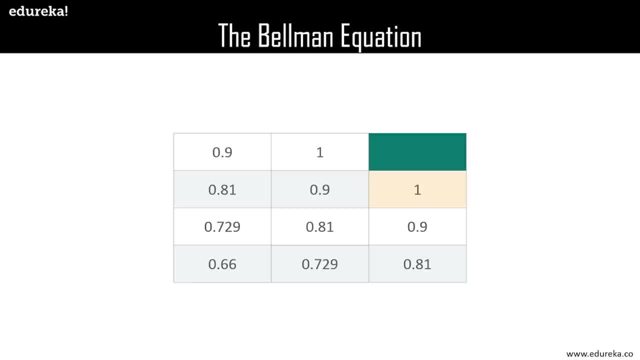 arbitrary room in the given location. now, if a robot lands up in the highlighted sky blue area, it will still feel the value of being in the green room if it stops at any arbitrary room in the given location. now, if a robot lands up in the highlighted sky blue area, it will. 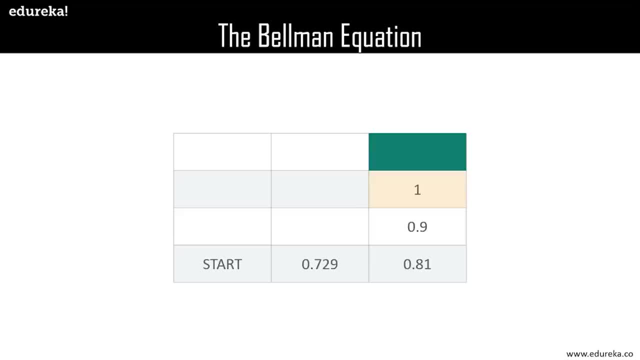 and then we again reach the starting point. so this is how the table looks, with some value footprints computed from the Bellman equation. now, a couple of things to notice here is that the max function helps the robot to always choose the state that gives it the maximum value of being in that state. now 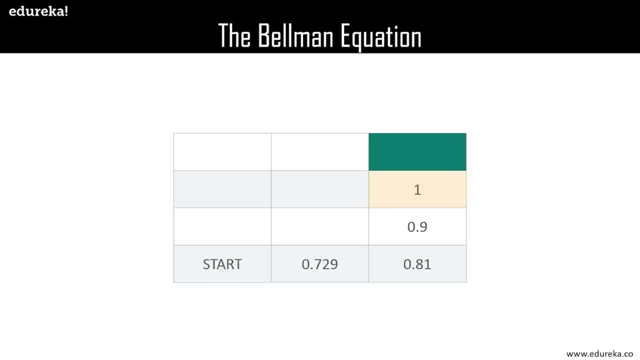 the discount factor gamma notifies the robot about how far it is from the destination. this is typically specified by the developer of the algorithm that would be installed in the robot. now, the other states can also be given their respective values in a similar way. so, as you can see here the boxes adjacent to 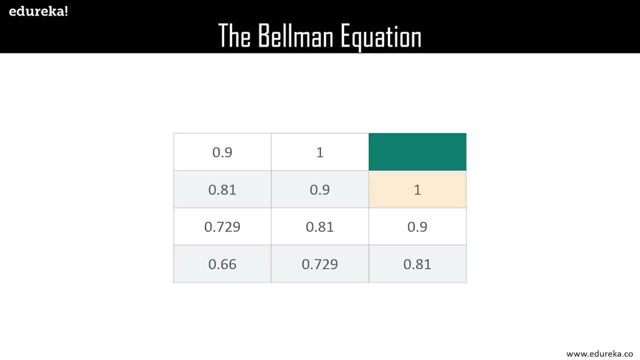 the green one, have one, and if we move away from one, we get 0.9, 0.81, 0.729 and finally we reach 0.66. now the robot now can proceed its way through the green room utilizing these value footprints, even if it's dropped at any arbitrary. 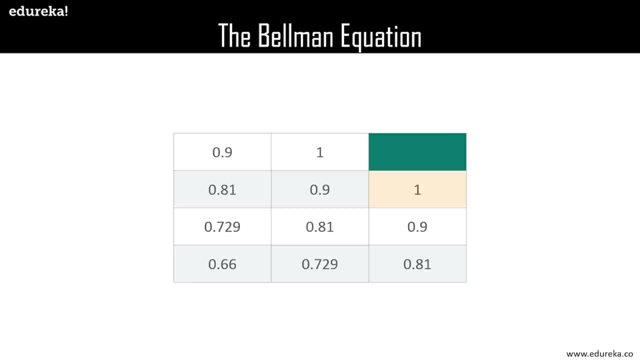 room in the given location. now, if a robot lands up in the highlighted sky blue area, it will still find two options to choose from, but eventually either of the paths will be good enough for the robot to take because of the way the value footprints are now laid out. now, one thing to note here is that the Bellman equation is one. 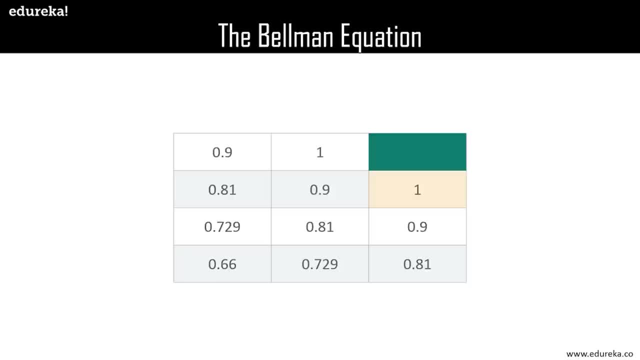 of the key equations in the world of reinforcement learning and Q learning. so, if we think realistically, our surroundings do not always work in the way we expect. there is always a bit of structure and a lot of things that we need to be aware of in order to be able to. 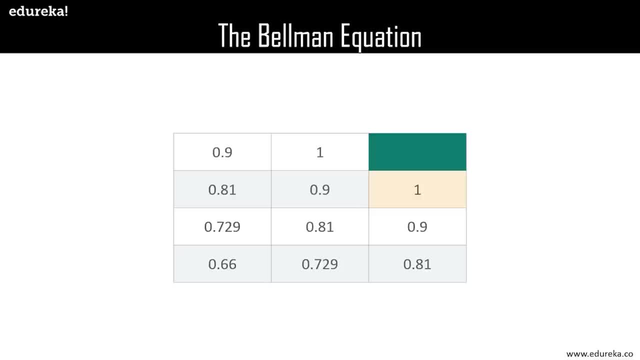 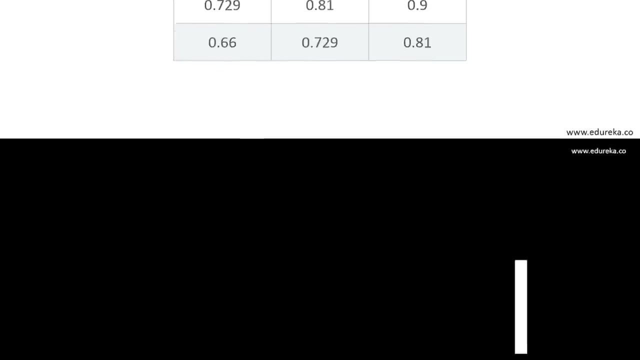 hair, the对ța בاؤv DVD's with proper in our case. now here comes the Markov decision process. but consider, the robot is currently in the red room and it's not one that has the fullным ability to rely on it. for so here comes the Markov decision process. the 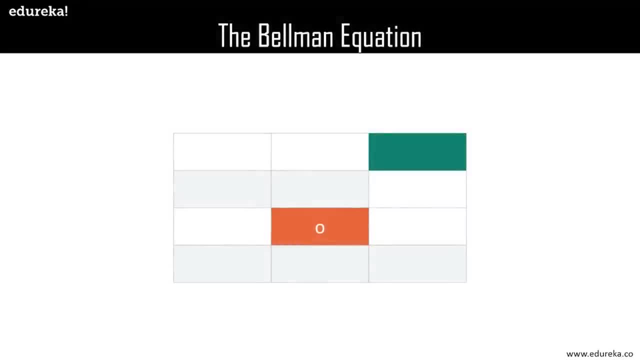 plot goes like this: the robot is leaving the room and safety comme ca, it needs to go to the green room now. let's now consider: the robot has a slight chance of dysfunctioning and might take the left or the right or the bottom turn instead of taking the. 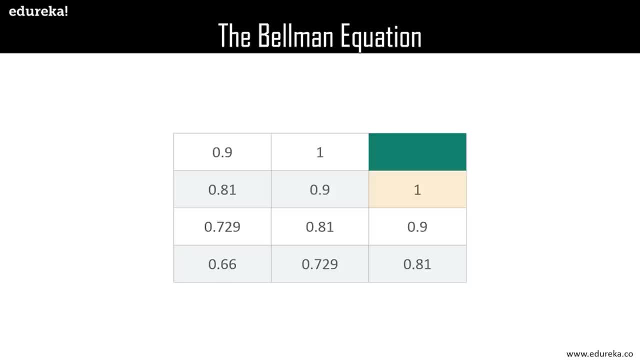 still find two options to choose from, but eventually either of the paths will be good enough for the robot to take because of the way the value footprints are now laid out. now, one thing to note here is that the bellman equation is one of the key equations in the world of reinforcement. 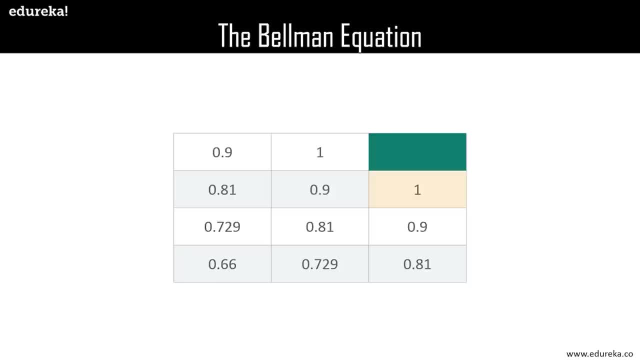 learning and q learning. so, if we think realistically, our surroundings do not always work in the way we expect. there is always a bit of stochasticity involved in it, but this applies to robot as well. sometimes it might be a little bit more complicated, and sometimes it might be a little bit more complicated. 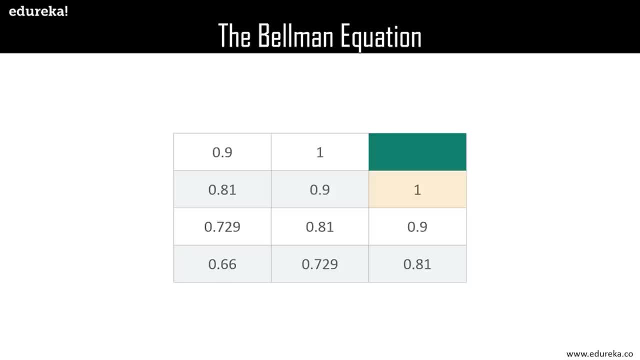 so happen that the robot's machinery got corrupted. sometimes the robot may come across some hindrance on its way which may not be known to it beforehand. right and sometimes, even if the robot knows that it needs to take the right turn, it will not. so how do we introduce the stochasticity in our case? 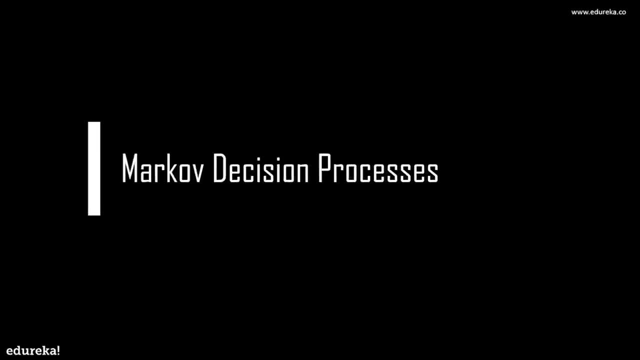 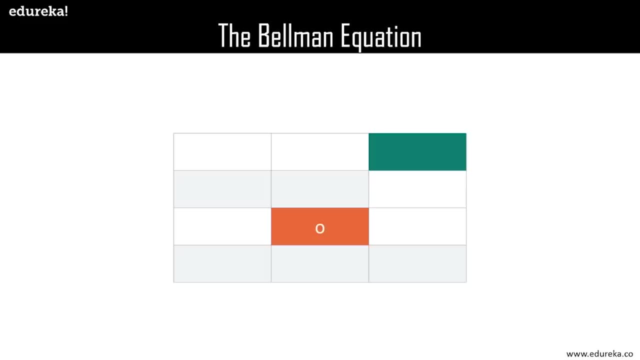 now here comes the mark of decision process. now consider: the robot is currently in the red room and it needs to go to the green room now. let's now consider the robot has a slight chance of dysfunctioning and might take the left or the right or the bottom turn instead. 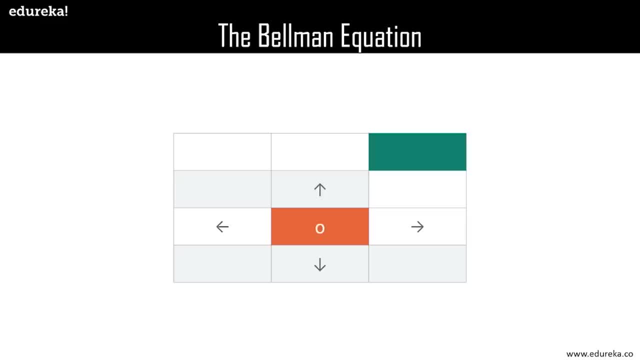 of taking the upper turn in order to get to the green room from where it is now, which is the red room. now the question is: how do we enable the robot to handle this when it is out in the given environment right now? this is a situation where the decision making regarding which turn is to 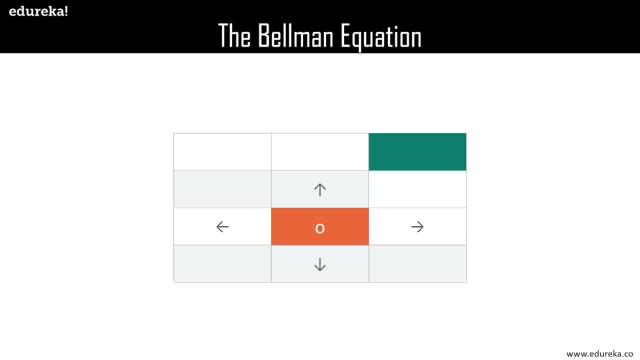 be taken is partly random and partly under the control of the robot. now. partly random because we are not sure when exactly the robot is going to take the right turn and the robot is going to take the left turn, exactly the robot might dysfunctional. and partly under the control of the robot because 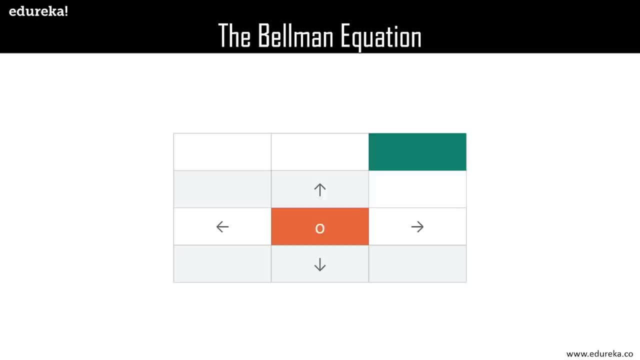 it is still making a decision of taking a turn right, on its own and with the help of the program embedded into it. so a mark of decision process is a discrete time stochastic control process. it provides a mathematical framework for modeling decision making in situations where the outcomes 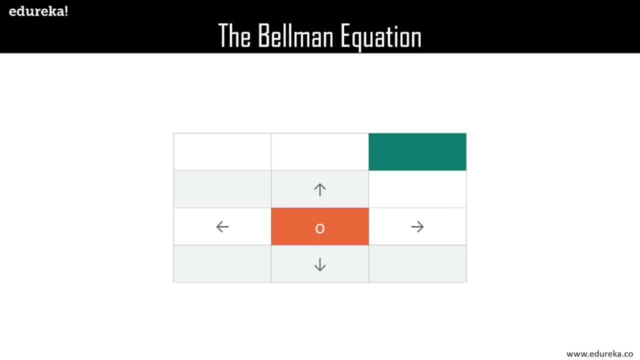 are partly random and partly under the control of the decision maker. now we need to give this concept a mathematical shape, most likely a mathematical shape, which is a mathematical shape, which is an equation which then can be taken further. now you might be surprised that we can do. 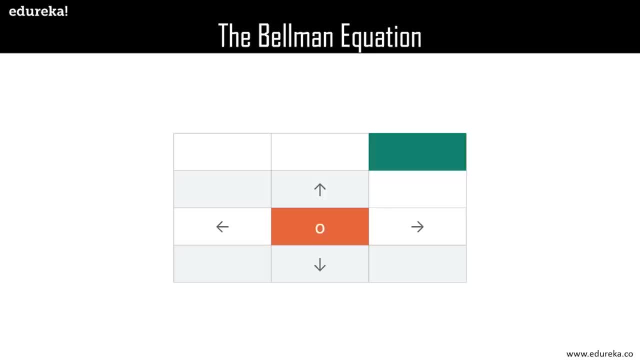 upper turn in order to get to the green room from where it is now, which is the red room. now the question is: how do we enable the robot to handle this when it is out in the given environment right now? this is a situation where the decision making regarding which turn is to be taken. 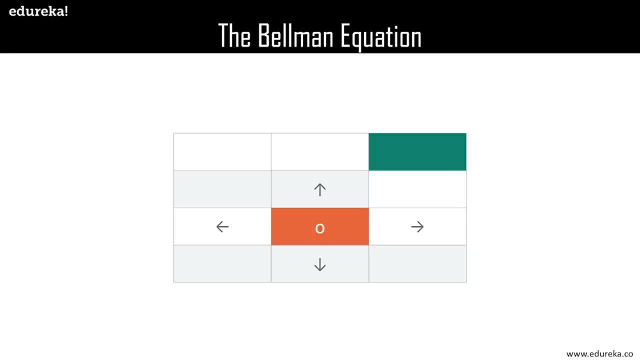 is partly random and partly under the control of the robot. now. partly random because we are not sure when exactly the robot might dysfunctional. and partly under the control of the robot because it is still making a decision of taking a turn right on its own and with the help of the program. 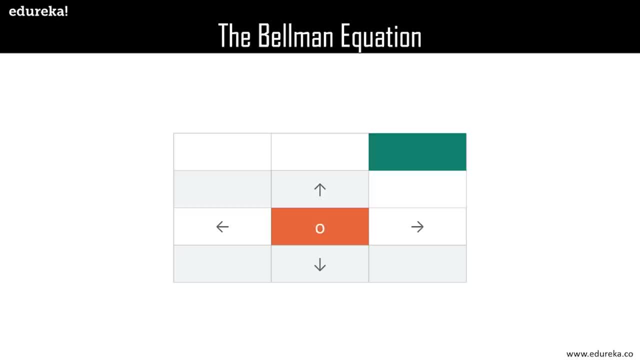 embedded into it. so a markov decision process is a discrete time stochastic control process. it provides a mathematical framework for modeling decision making in situations where the outcomes are partly random and partly under the control of the robot. so a markov decision process is a random and partly under the control of the decision maker. now we need to give this concept. 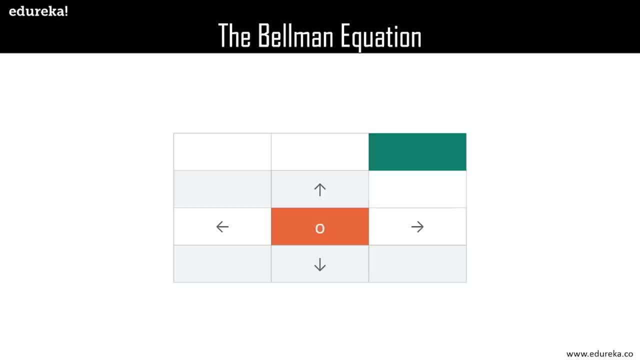 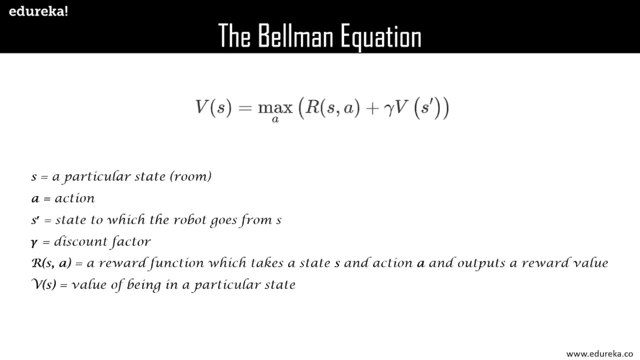 a mathematical shape, most likely an equation, which then can be taken further. now you might be surprised that we can do this with the help of the bellman equation, with a few minor tweaks. so if we have a look at the original bellman equation, v of x is equal to maximum of r, s, comma, a plus gamma v. 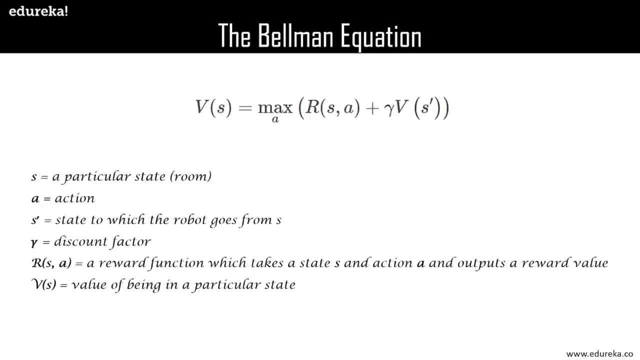 of s dash. what needs to be changed in the above equation so that we can introduce some amount of randomness here? as long as we are not sure when the robot might not take the expected turn, we are then also not sure in which room it might end up, in which is nothing but the room it. 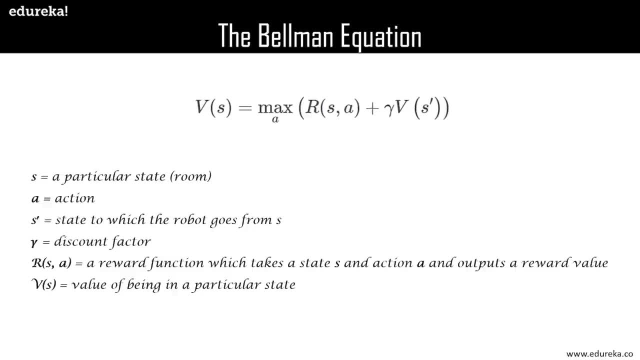 moves from its current room. at this point, according to the equation, we are not sure of the s dash, which is the next state or the room, but we do know all the probable turns the robot might take. now, in order to incorporate each of those probabilities into the above equation, we need to know the probability of the robot taking the next turn. 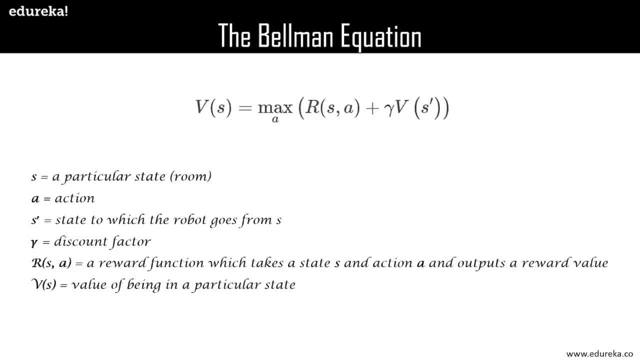 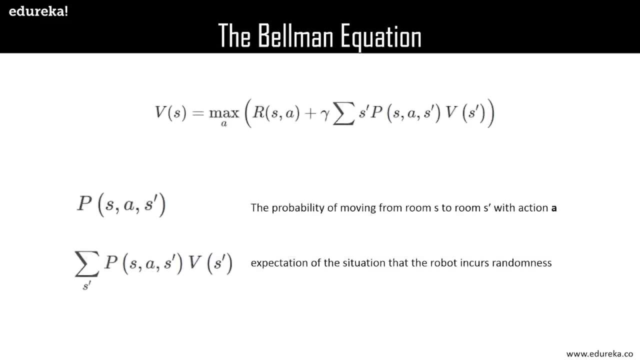 we need to associate a probability with each of the turns to quantify the robot if it has got any explicit chance of taking this turn now. if we do so, we get p? s is equal to maximum of r s comma a plus gamma. into summation of s dash: p s comma a comma s dash into v of s dash, now the p s, a and s. 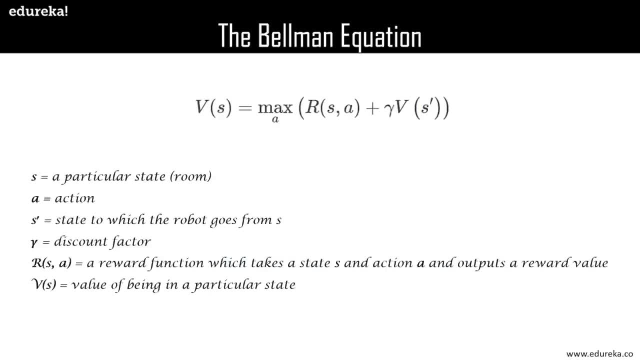 this with the help of the bellman equation, with a few minor tweaks. so if we have a look at the original bellman equation, v of x is equal to maximum of r, s comma a plus gamma v of s dash. what needs to be changed in the above equation so that we can introduce some amount of randomness? 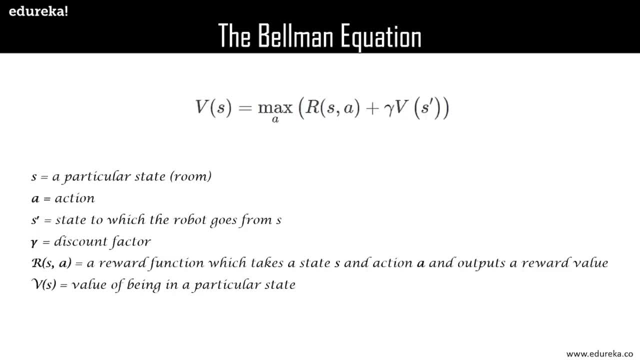 here. as long as we are not sure when the robot might not take the expected turn, we are then also not sure in which room it might end up in, which is nothing but the room it moves from its current room. at this point, according to the equation, we are not sure of the s dash, which is the next state. 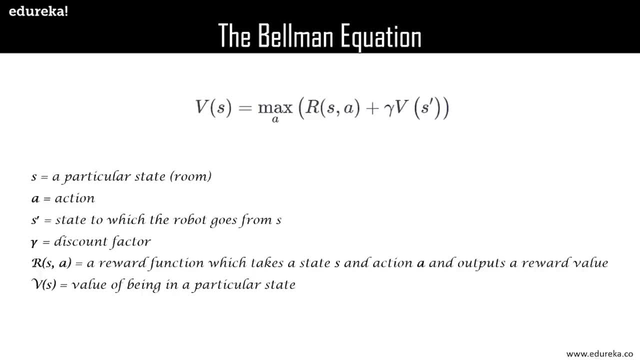 or the room, but we do know all the probable turns the robot might take. now, in order to incorporate each of those probabilities into the above equation, we need to associate a probability with each of the turns to quantify the robot: if it has a probability of x and y and if it has a probability of y and if it has a probability of y, and. 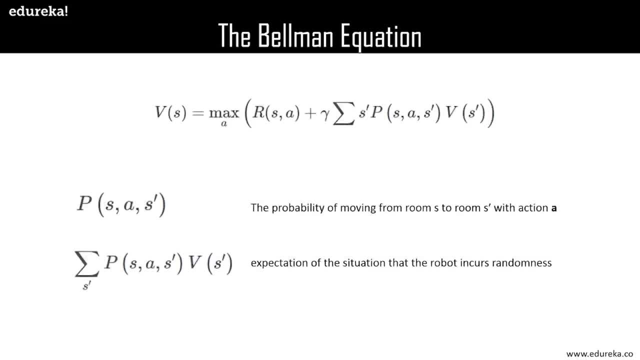 got any explicit chance of taking this turn now. if we do so, we get: PS is equal to maximum of R, s comma a plus gamma into summation of s dash, P s comma a comma s dash into V of s dash. now the PS a and s dash is the probability of. 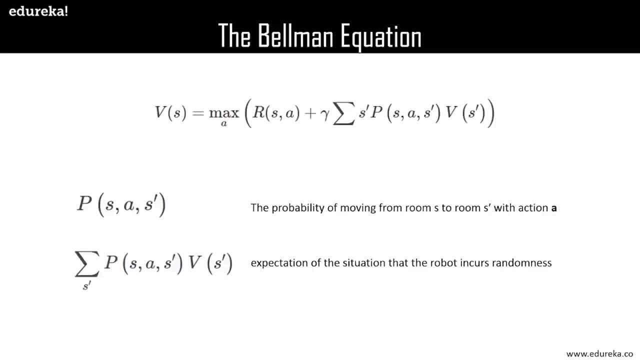 moving from room s to s dash with the action a, and the submission here is the expectation of the situation that the robot incurs, which is the randomness now let's take a look at this example here. so when we associate the probabilities to each of these turns, we essentially mean that there is an 80% chance that 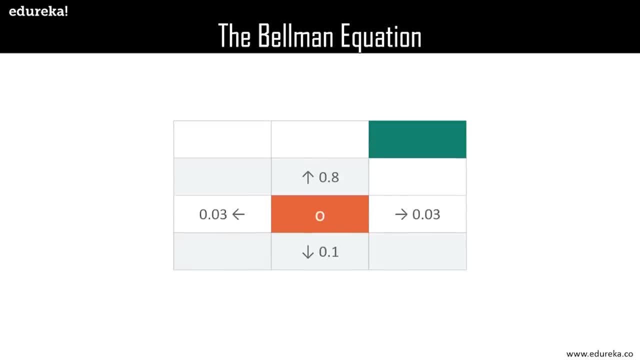 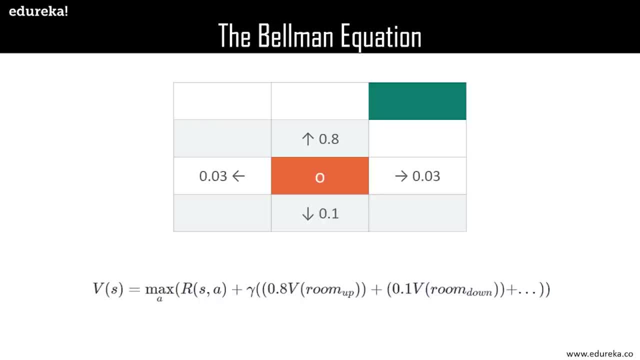 0.8 into V of room up plus 0.8 into V of room up plus 0.8 into V of room up plus 0.1 into V of room down, 0.03 into room of V of room left plus 0.03 into V of. 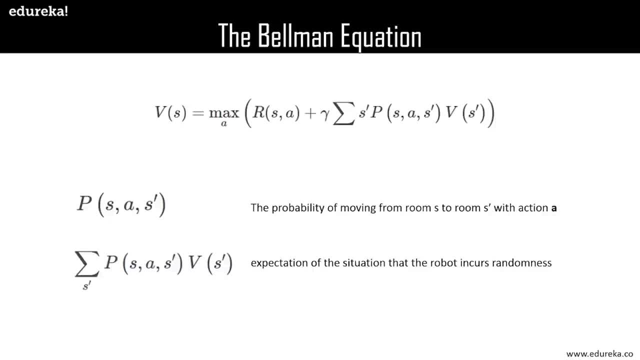 dash is the probability of moving from room s to s dash. so we need to associate a probability with the action a, and the summation here is the expectation of the situation that the robot incurs, which is the randomness. now let's take a look at this example here. so when we associate 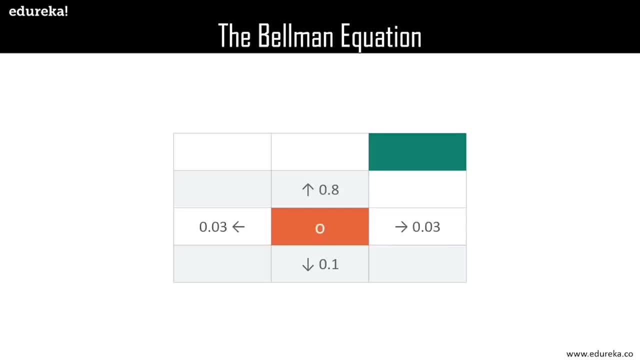 the probabilities to each of these turns. we essentially mean that there is an 80 chance that the robot will take the upper turn. now, if we put all the required values in our equation, we get: v of s is equal to maximum of r of s, comma a plus gamma. 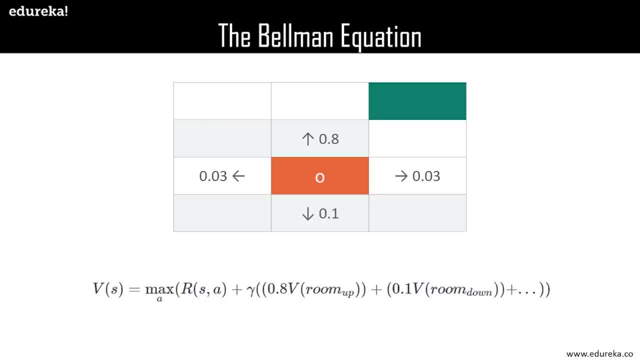 of 0.8 into v of room up plus 0.1 into v of room down, 0.03 into room of v of room left plus 0.03 into v of room right now. note that the value footprints will not change due to the fact that 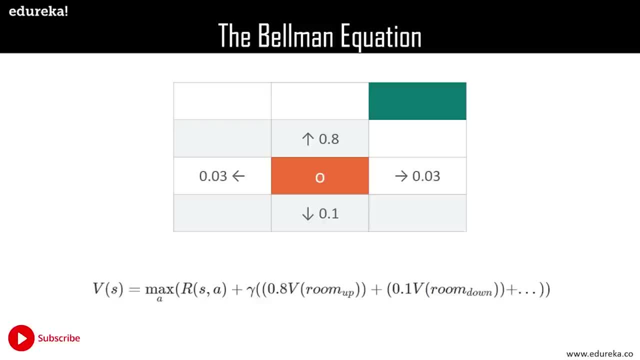 we are incorporating stochastically here, but this time we will not calculate those value footprints. instead we will let the robot to figure it out. now, up until this point, we have not considered about rewarding the robot with the value footprints. we have not considered about rewarding the robot with 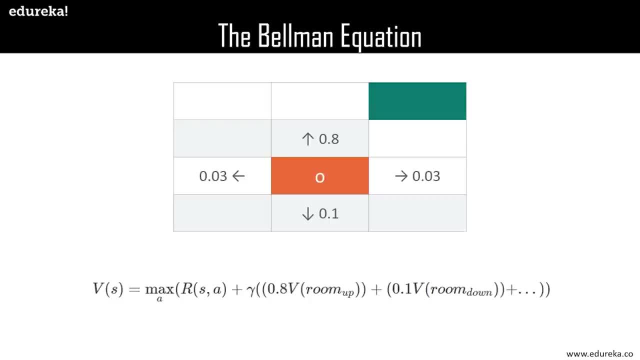 for its action of going into a particular room. we are only rewarding the robot when it gets to the destination. now, ideally, there should be a reward for each action the robot takes to help it better assess the quality of the actions. but the rewards need not to be always be the same, but it is much. 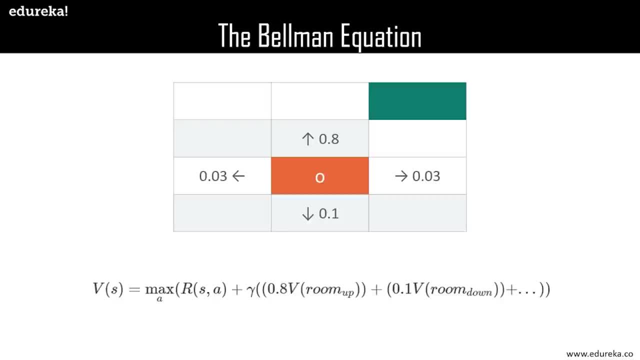 better than having some amount of reward for the actions than having no rewards at all. right, and this idea is known as the living penalty. in reality, the reward system can be very complex, and particularly modeling sparse rewards is an active area of research in the domain of reinforcement learning. so by now we have got the equation which we have. so what? 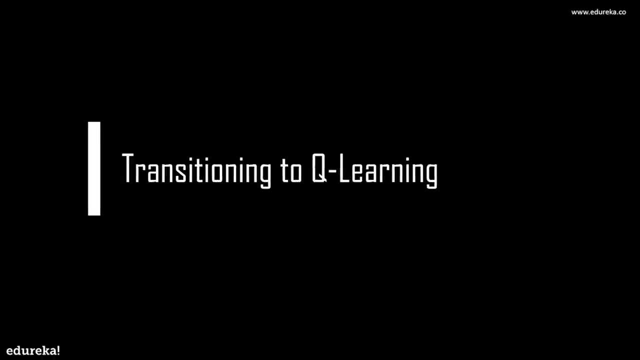 we're going to do is now transition to q learning. so this equation gives us the value of going to a particular state, taking the stochasticity of the environment into account. now we have also learned, very briefly, about the idea of living penalty, which deals with associating each move of the 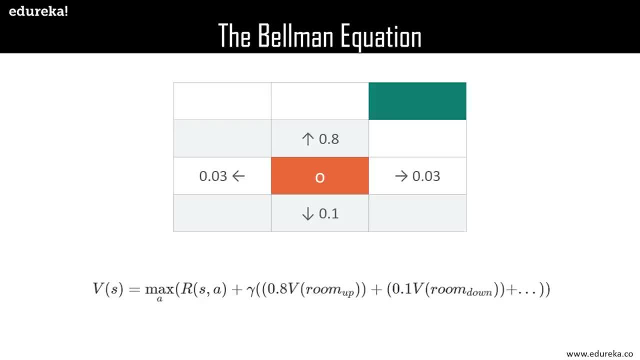 room right now. note that the value footprints will not change due to the fact that we are incorporating stochastically here, but this time we will not calculate those value footprints. instead, we will let the robot to figure it out. now, up until this point, we have not considered about rewarding. 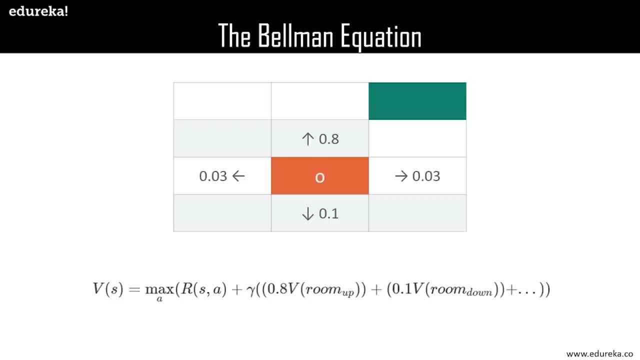 the robot for its action of going into a particular room. we are only rewarding the robot when it gets to the destination. now, ideally, there should be a reward for each action the robot takes to help it better assess the quality of the actions. but the rewards need not to be always be the same, but it is much. 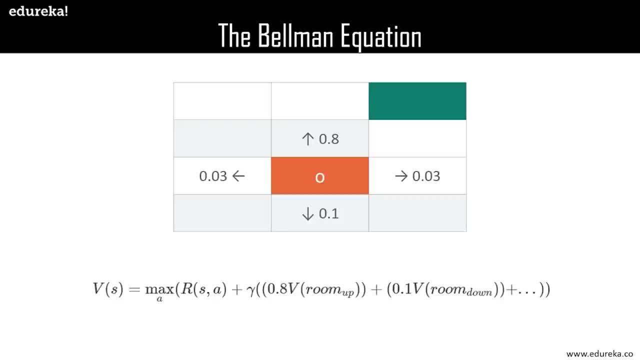 better than having some amount of reward for the actions than having no rewards at all. right, and this idea is known as the living penalty. in reality, the reward system can be very complex, and particularly modeling sparse rewards is an active area of research in the domain of reinforcement learning. so by now we 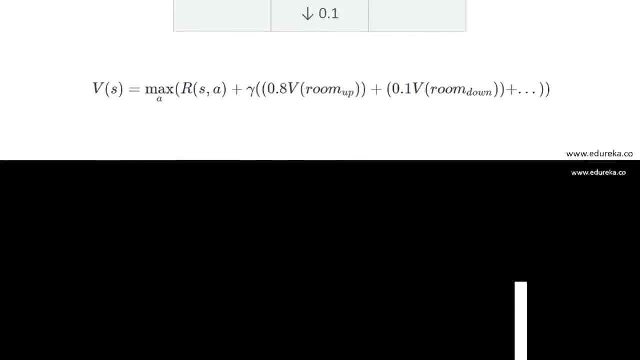 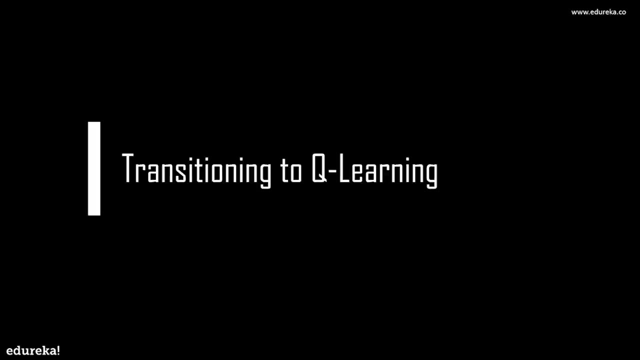 have got the equation. which we have is. so what we're going to do is now transition to Q learning. so this equation gives us the value of going to a particular state, taking the stochasticity of the environment into account. now we have also learned very briefly about the idea of living. 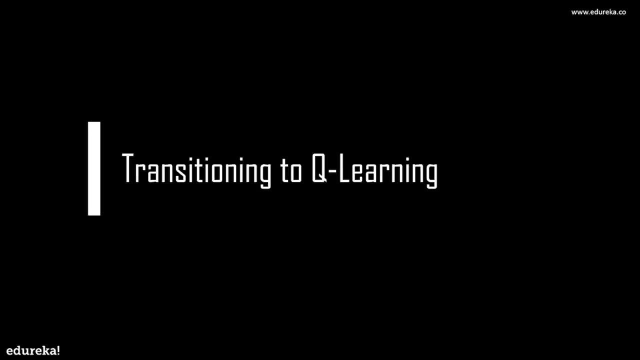 penalty, which deals with associating each move of the robot with a reward. so Q learning possesses an idea of assessing the quality of an action that is taken to move to a state and rather than determining the possible value of the state which is being moved to, so earlier. 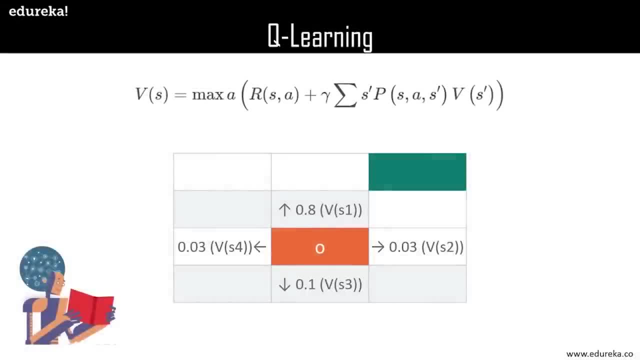 we had 0.8 into V of s1, 0.03 into V of s2, 0.1 into V of s3, and so on. now, if we incorporate the idea of assessing the quality of the action for moving to a certain state, so the environment with the agent and the quality of the action, 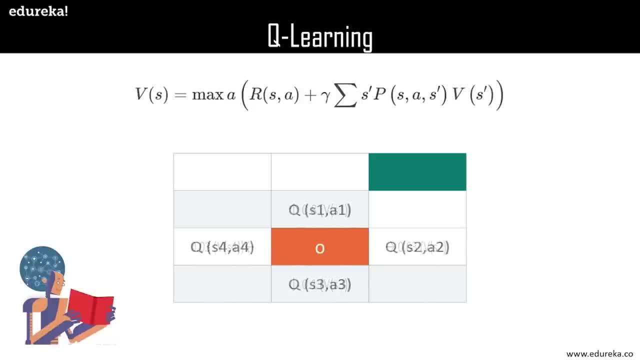 will look something like this. so instead of 0.8 V of s1, we'll have Q of s1 comma a1, we'll have Q of s2 comma a2, Q of s3. now the robot now has four different states to choose from and along. 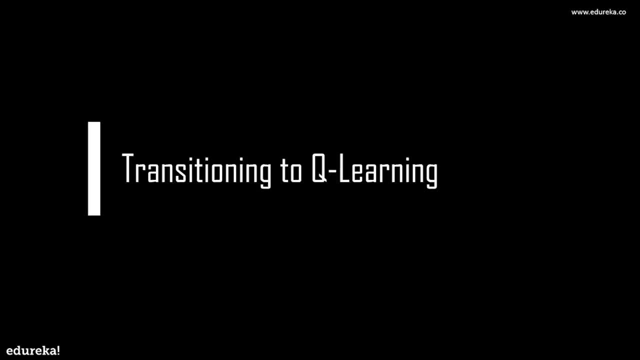 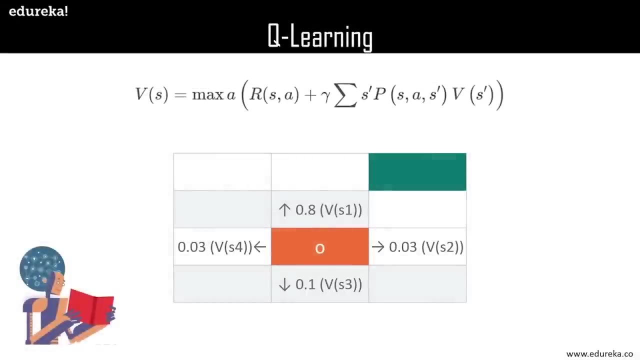 robot with a reward. so q learning possesses an idea of assessing the quality of an action that is taken to move to a state, rather than determining the possible value of the state which is being moved to. so earlier we had 0.8 into v of s1, 0.03 into v of s2, 0.1 into v of s3, and so on. now, if we incorporate the idea, 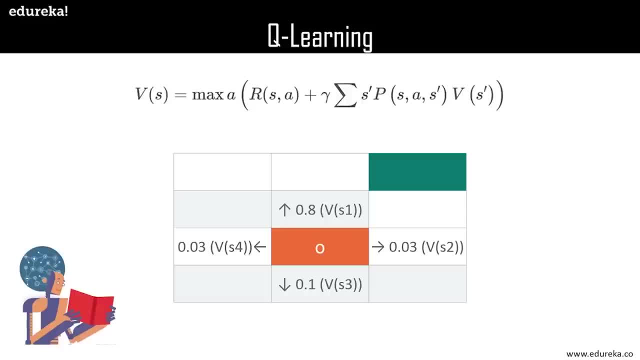 of assessing the quality of the action for moving to a certain state, so the environment, the agent and the quality of the action will look something like this: so instead of 0.8 v of s1 will have q of s1, comma a1 will have q of s2, comma a2, q of s3. now the robot now has four different states. 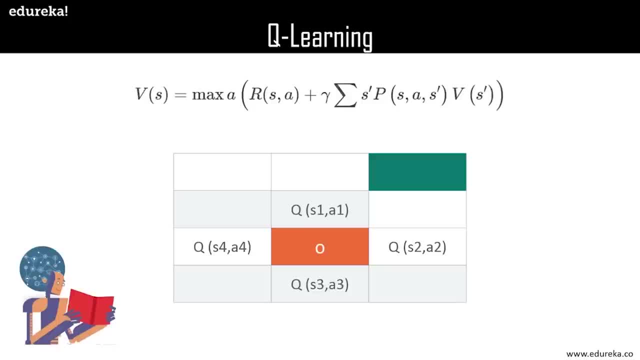 to choose from, and along with that there are four different actions, also for the current state it is in. so how do we calculate q of s comma a? that is the cumulative quality of the possible actions the take. so let's break it down now from the equation: v of s equals maximum of a r s comma, a plus comma. 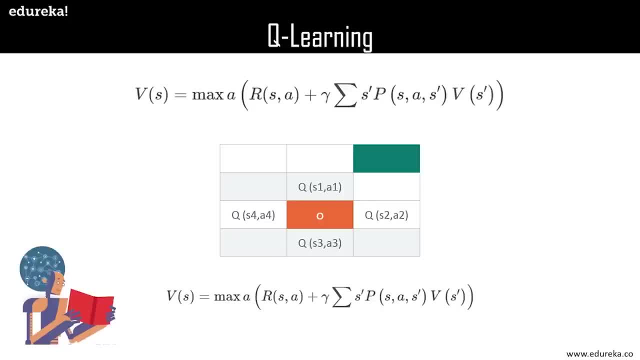 summation s dash, p s, a s dash into v of s dash. if we discard the maximum function, we have r? s of a plus gamma into summation p and v. now, essentially, in the equation that produces v of s, we are considering all possible actions and all possible states from the current state that the 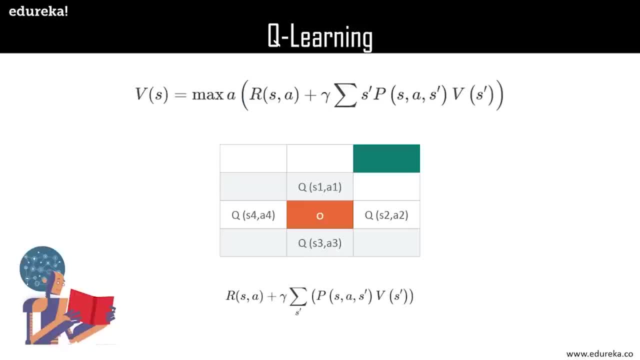 robot is in and then we are taking the maximum value caused by taking a certain action and the equation produces a value footprint which is for just one possible action. in fact we can think of it as the quality of the action. so q of s comma a is equal to r s comma a plus comma of summation. 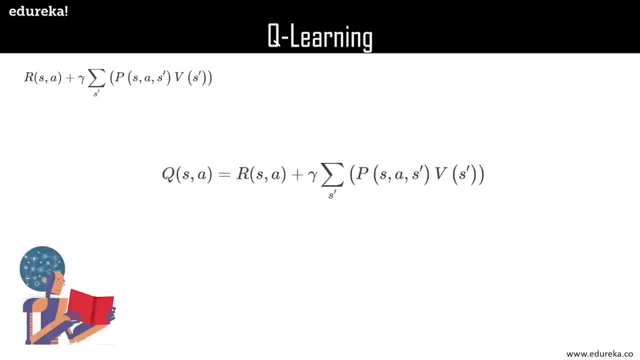 p and v. now that we have got an equation to quantify the quality of a particular action, we are going to make a little adjustment in the equation. we can now say that v of s is the maximum of all the possible values of q of s comma a right. so let's utilize this fact and replace v of s dash as a function of q. 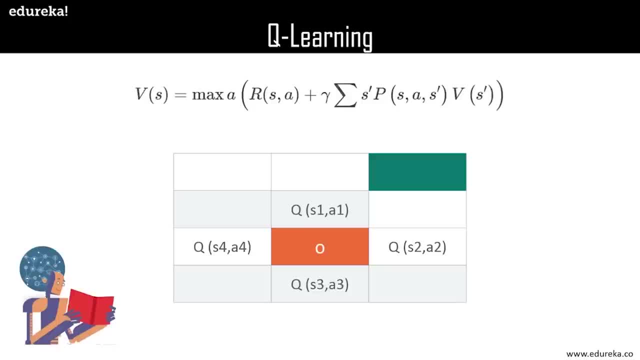 with that there are four different actions, also for the current state it is in. so how do we calculate Q of s comma a? that is the cumulative quality of the possible actions the robot might take. so let's break it down now from the equation we: V of S equals maximum of A, R, S comma A plus comma summation S dash, P, S, A, S dash into V of S dash. 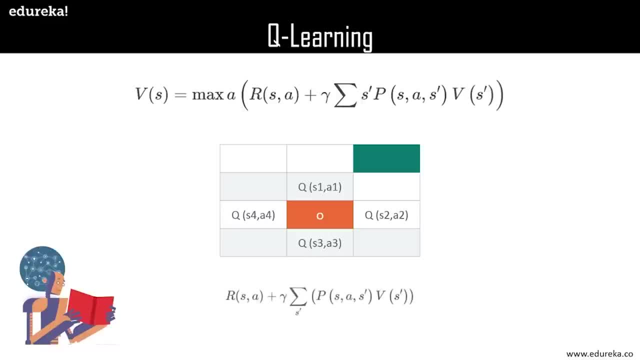 If we discard the maximum function, we have R S of A plus gamma into summation P and V. Now, essentially, in the equation that produces V of S, we are considering all possible actions and all possible states from the current state that the robot is in, and then we are taking the maximum. 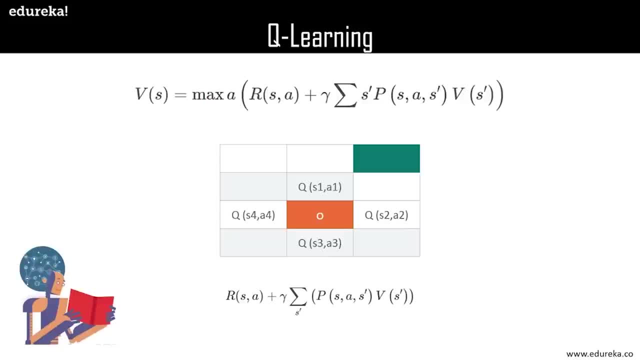 value caused by taking a certain action, and the equation produces a value footprint which is for just one possible action. In fact we can think of it as the quality of the action. So Q of S comma A is equal to R S comma A plus gamma of summation P and V. Now that we have got an equation to quantify. 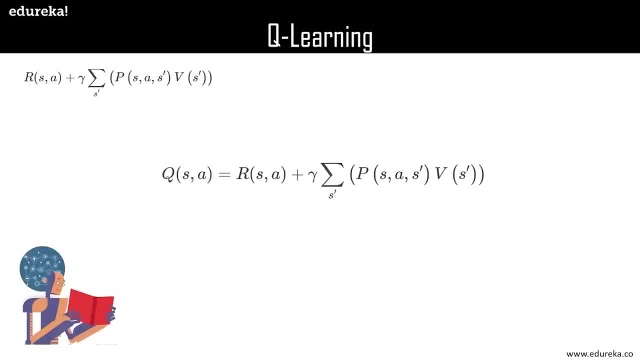 the quality of a particular action. we are going to make a little adjustment in the equation. We can now say that the value of the action is equal to the value of the action. So Q of S comma A is the maximum of all the possible values of Q of S comma A. right, So let's utilize this fact and 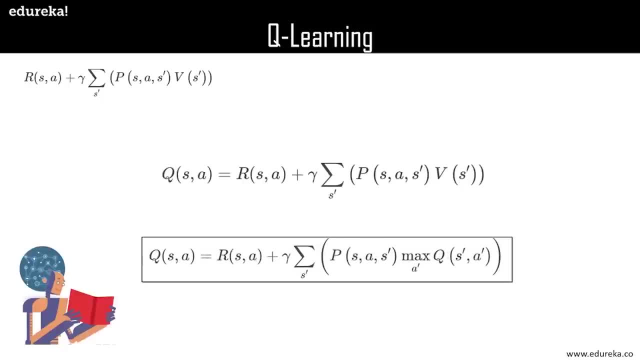 replace V of S dash as a function of Q. So Q S comma A becomes R of S comma A, plus comma of summation, P S A S dash and maximum of the Q S dash A dash. So the equation of V is now turned into an equation of Q, which is the quality. 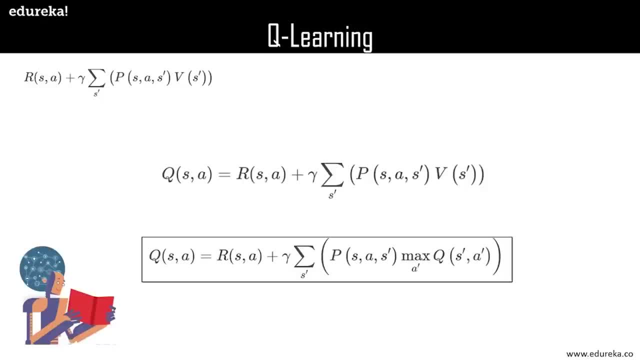 But why would we do that Now? this is done to ease our calculations, because now we have only one function, Q, which is also the core of the dynamic programming language. We have only one function, Q, to calculate, and R of S comma A is a quantified metric which produces reward of moving to a certain 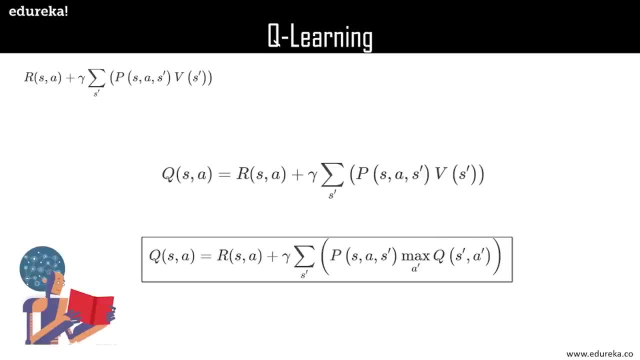 state. Now the qualities of the actions are called the Q values, and from now on we will refer to the value footprints as the Q values. Now, the second piece of the puzzle is the temporal difference. Now, temporal difference is the component that will help the robot calculate the Q values with respect to the changes in the environment. 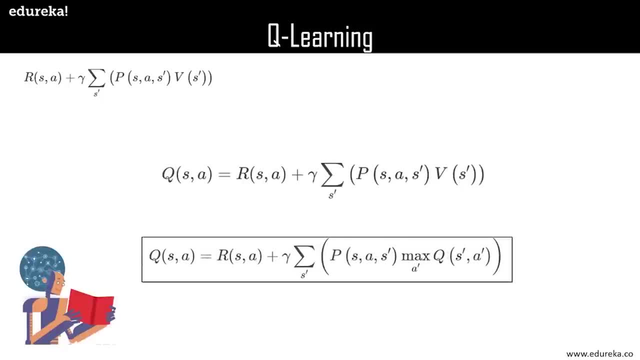 so q s comma a becomes r of s comma a, plus comma of summation, p s a s dash and maximum of the q s dash a dash. so the equation of v is now turned into an equation of q, which is the quality. but why would we do that now? this is done to ease our calculations. 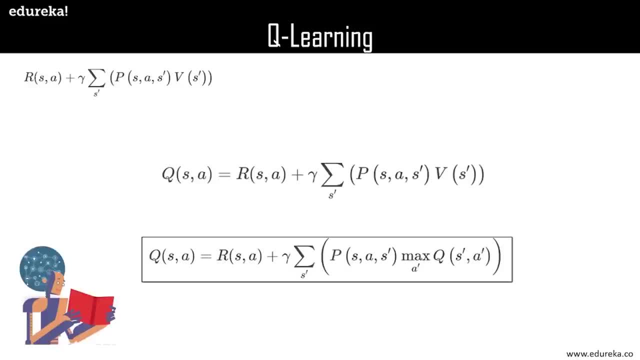 because now we have only one function, q, which is also the core of the dynamic programming language. we have only one function, q to calculate, and r of s comma a is a quantified metric which produces reward of moving to a certain state. now the qualities of the actions are called the q. 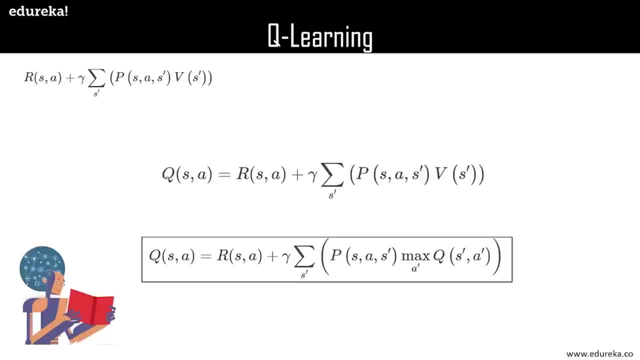 values and from now on we will refer to the value footprints as the q values. an important piece of the puzzle is the temporal difference. now, temporal difference is the component that will help the robot calculate the q values with respect to the changes in the environment over time. so consider: our robot is currently in the 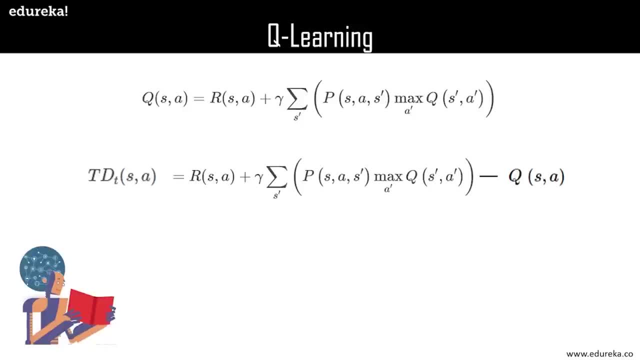 marked state and it wants to move to the upper state. one thing to note that here is that the robot already knows the q value of making the action that is moving to the upper state, and we know that the environment is stochastic in nature and the reward that the robot will get after moving to the upper state might be different. 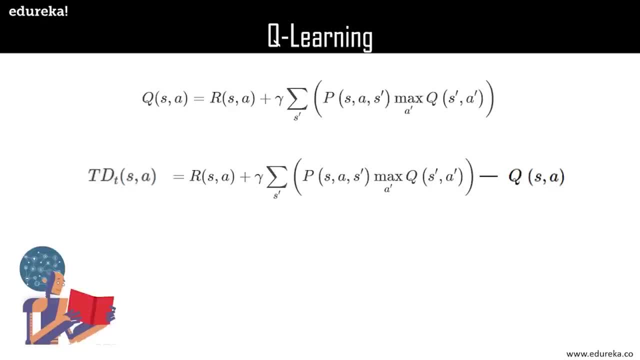 from an earlier observation. so how do we capture this change, the real difference? we calculate the new q s, comma a with the same formula and subtract the previously known q s a from it. so this will in turn give us the new qa. now, the equation that we just derived gives the temporal difference. 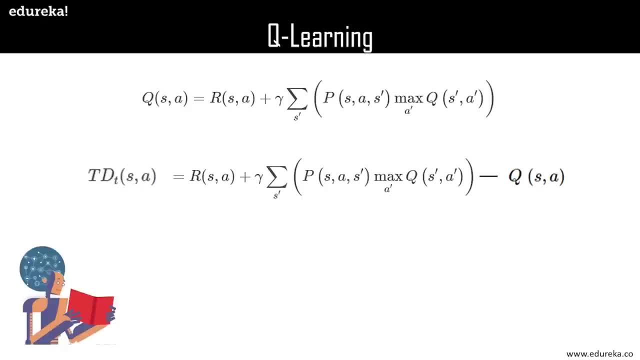 in the q values, which further helps to capture the random changes in the environment over time. so the new qs, comma a is the positive prompt at this point. it is the new qa which is the new qa at this point and means the qa in this particular case, which is now in the, the current. 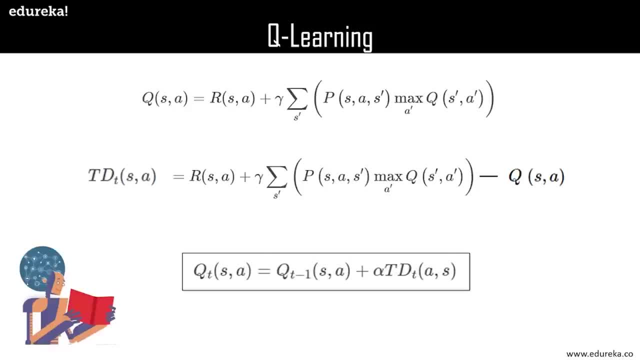 state, which is the environment which may impose. now the new q s comma a is updated as the following: so q t of s comma a is equal to q t minus one s comma a plus alpha d, d d of a comma s. now here, alpha is the learning rate, which controls how quickly the robot adapts to the random changes. 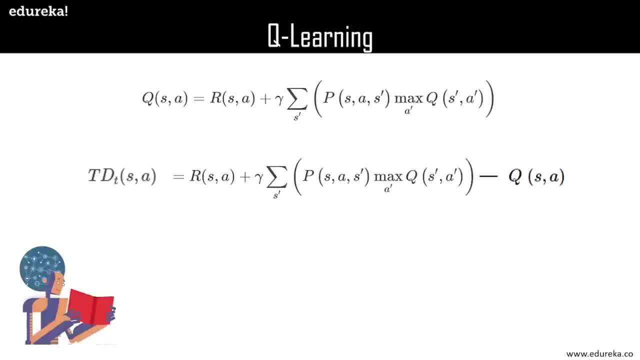 over time. So consider: our robot is currently in the marked state and it wants to move to the upper state. One thing to note that here is that the robot already knows the Q value of making the action that is, moving to the upper state, and we know that the environment is stochastic in nature. 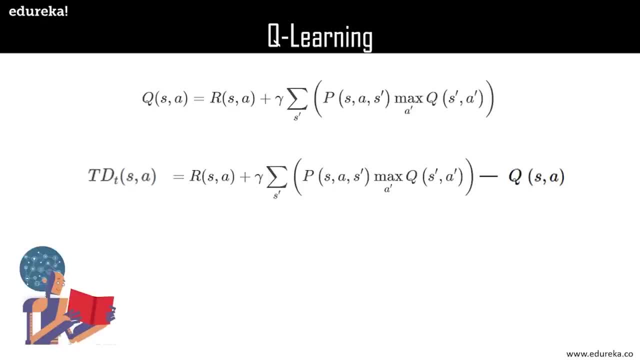 and the reward that the robot will get after moving to the upper state is the Q value of the action. So the new Q value of moving to the upper state might be different from an earlier observation. So how do we capture this change, the real difference? We calculate the new Q with the same. 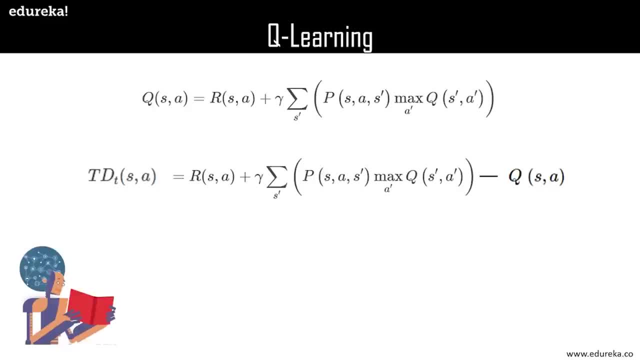 formula and subtract the previously known Q from it, So this will, in turn, give us the new Q. Now the equation that we just derived gives the temporal difference in the Q values, which further helps to capture the random changes in the environment which may impose Now the new Q. 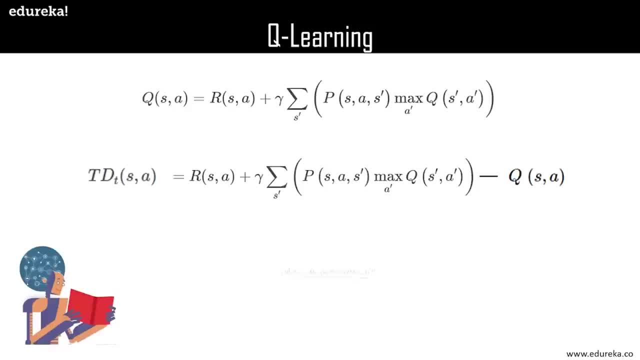 is updated as the following. So Qt of s comma a is equal to Qt minus 1 s comma a plus alpha tdt of a comma s. Now here alpha is the learning rate, which controls how quickly the robot adapts to the random changes imposed by the environment. The Qt s comma a is the current state Q value. 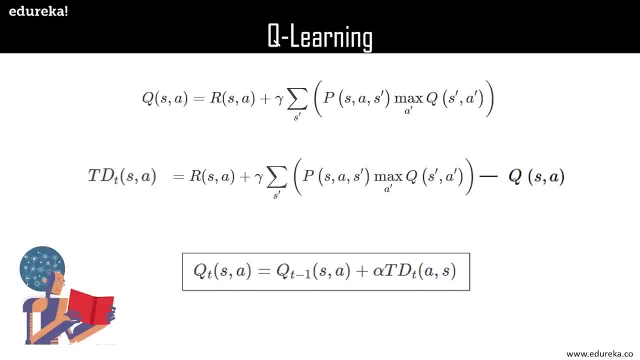 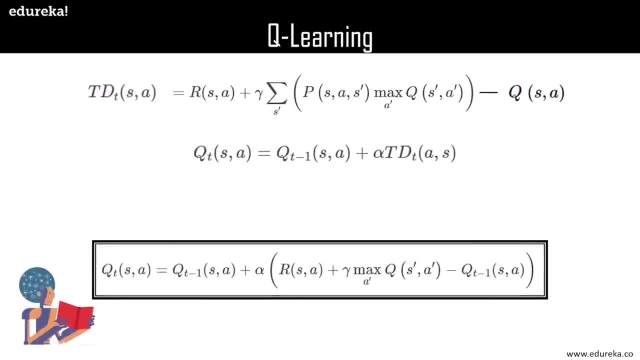 and the Qt minus 1 s comma a is the previously recorded Q value. So if we replace the tds comma a with its full form equation, we should get: Qt of s comma a is equal to Qt minus 1 of s comma a, plus alpha into r of s comma a plus gamma maximum of Q s dash, a dash minus Qt minus 1 s comma a. 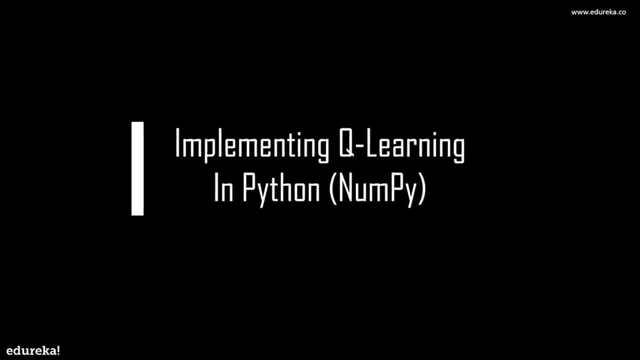 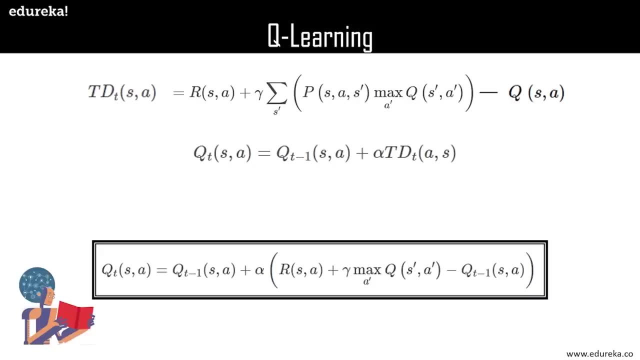 Now that we have all the little pieces of Q learning together, let's move forward to its implementation part. Now, this is the final equation of Q learning, right? So let's see how we can implement this And obtain the best path for any robot to take Now to implement the algorithm we need to. 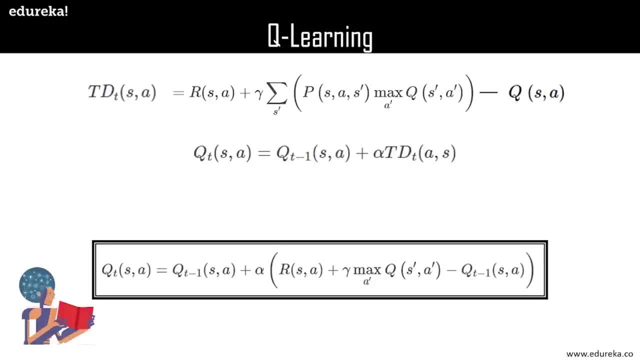 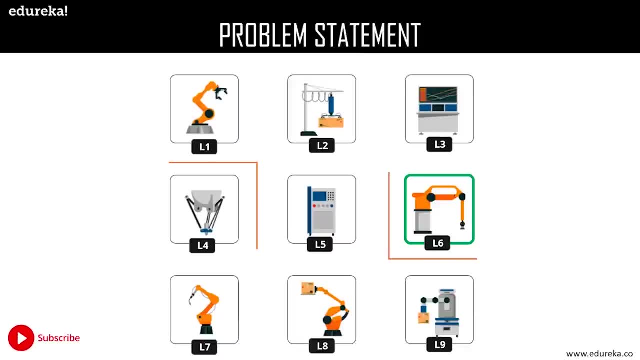 understand the warehouse location and how that can be mapped to different states. So let's start by recollecting the sample environment. So, as you can see, here we have L1, L2, L3 to L9.. And, as you can, 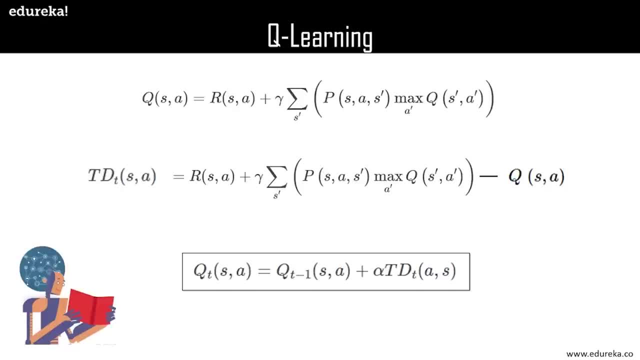 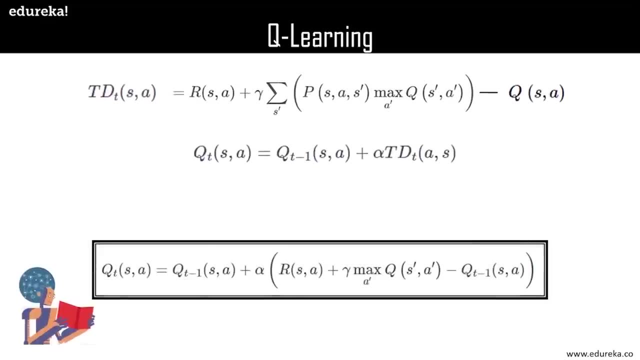 imposed by the environment. the q t s comma a is the current state q value and the q t minus one s value. So if you replace the TD s comma a with its full form equation, we should get: qt of s comma a is equal to qt minus 1 of s comma a plus alpha into r of s comma a plus gamma maximum of. 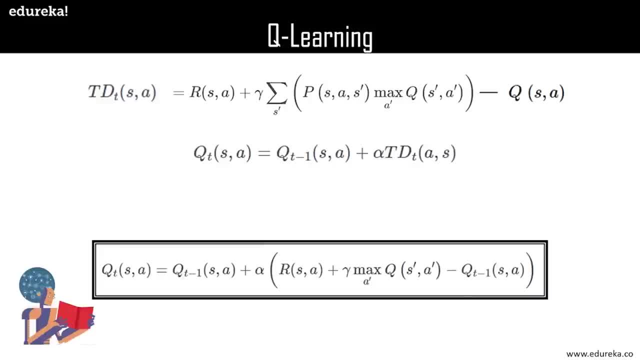 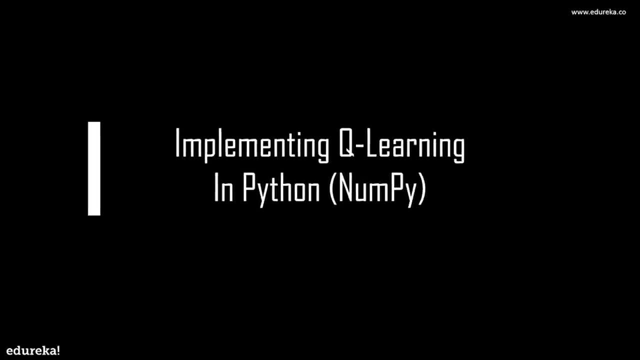 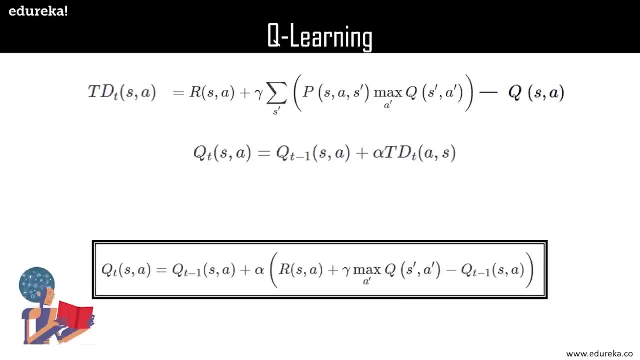 q s dash a, dash minus qt, minus 1 s comma a. Now that we have all the little pieces of q learning together, let's move forward to its implementation part. Now, this is the final equation of q learn right. So let's see how we can implement this and obtain the best path for any robot to take. 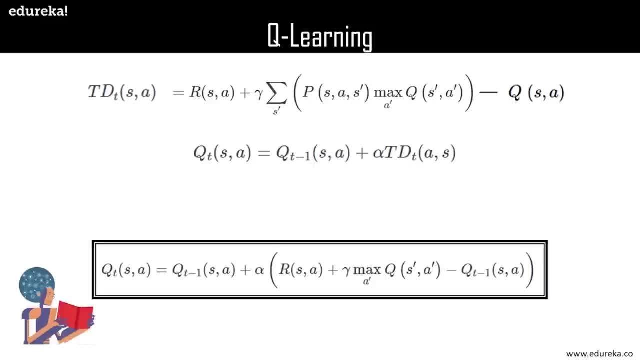 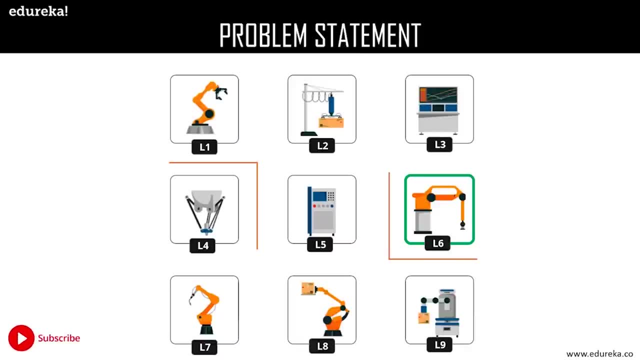 Now, to implement the algorithm, we need to understand the warehouse location and how that can be mapped to different states. So let's start by recollecting the sample environment. So, as you can see here we have L1, L2, L3 to L9 and, as you can see here we have certain borders. 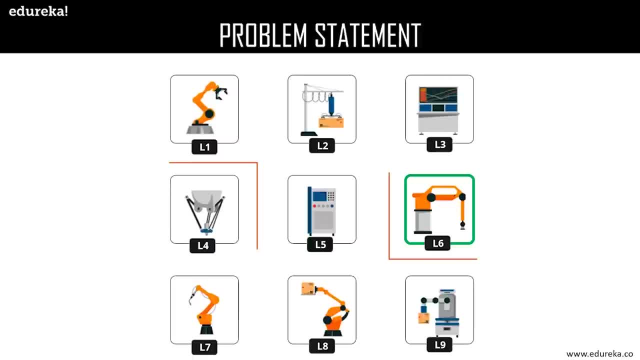 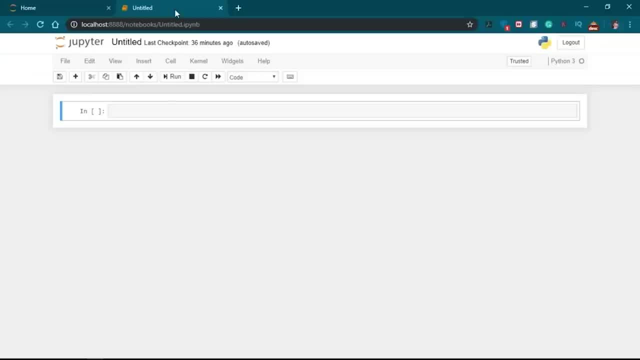 also. So, first of all, let's map each of the above locations In the warehouse to numbers are the states, so that it will ease our calculations right. So what I'm going to do is create a new Python 3 file in the Jupyter notebook, and I'll name it as: 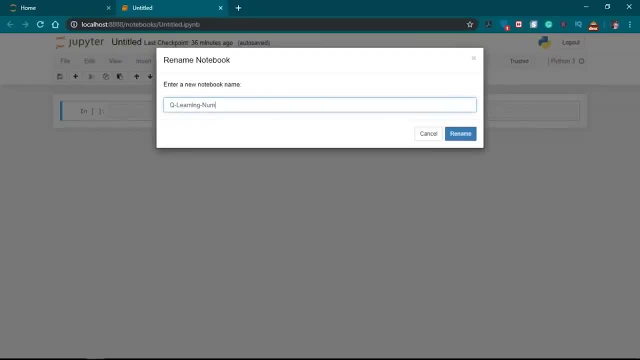 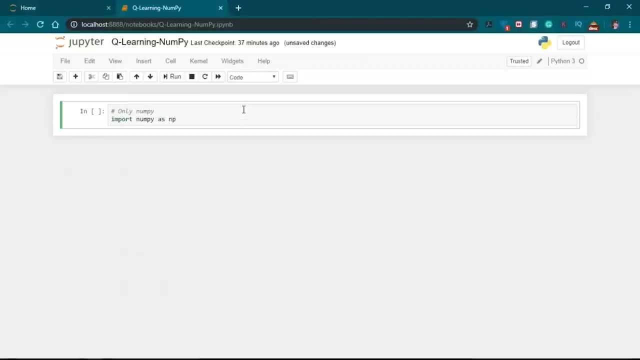 q learning numpy. Okay, so let's define the states, But before that, what we need to do is import numpy, because we're going to use numpy for this purpose, And let's initialize the parameters, that is, the gamma And alpha parameters. So gamma is 0.75,, which is the discount factor, whereas alpha is 0.9,. 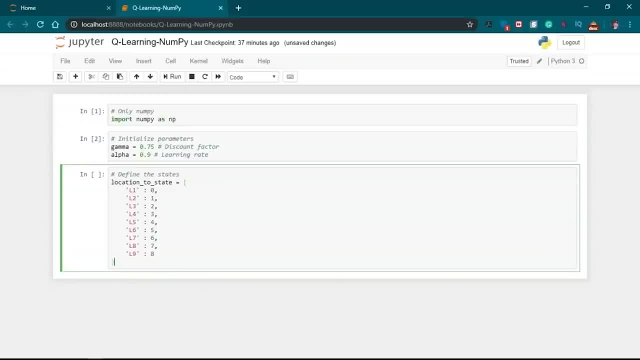 which is the learning rate. Now, next, what we're going to do is define the states and map it to numbers. So, as I mentioned earlier, L1 is 0 and till L9, we have defined the states in the numerical form. Now the next step is to define the actions, which is, as mentioned above, represent the 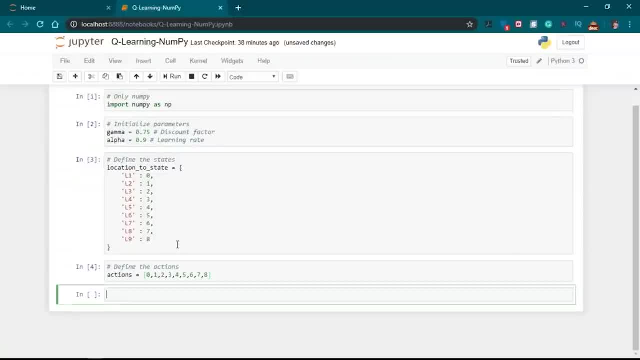 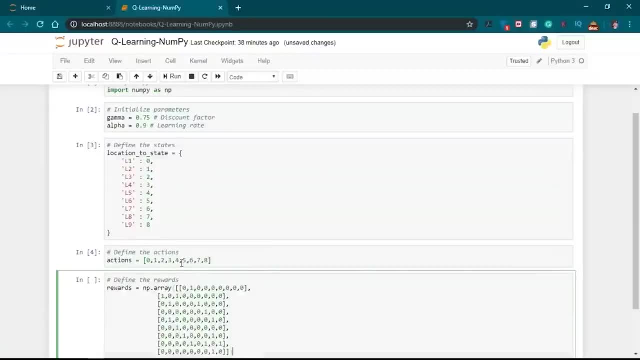 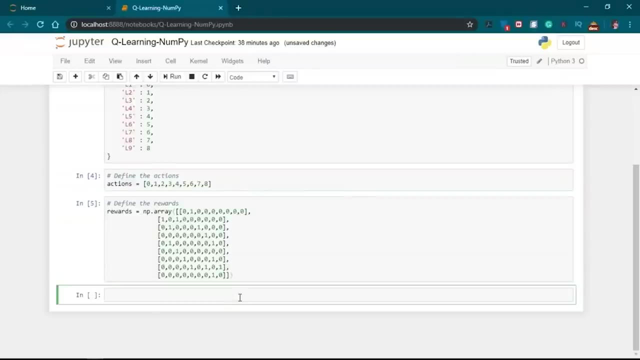 transition to the next state. So, as you can see, here we have an array of actions, from the 0 to 8.. Now what we're going to do is define the reward table. So, as you can see, it's the same matrix that we created just now, that I showed you just now. Now, if you understood it correctly, 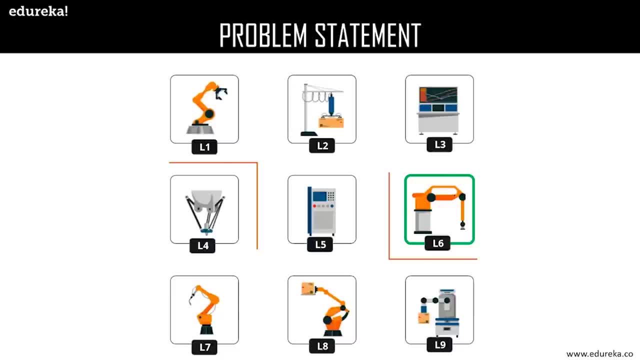 see, here we have certain borders also. So first of all, let's map each of the above locations in the warehouse to numbers or the states, so that it can be mapped to the different states. So let's use our calculations, right? So what I'm going to do is create a new Python 3 file in the Jupyter. 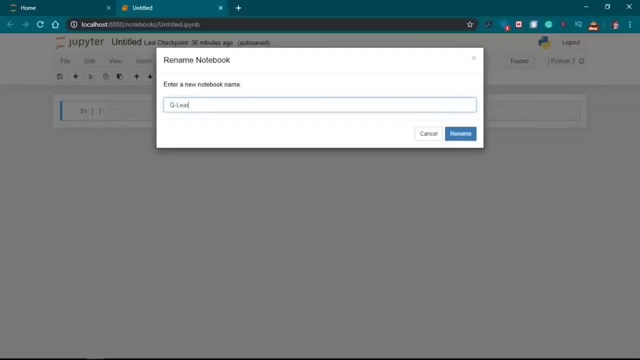 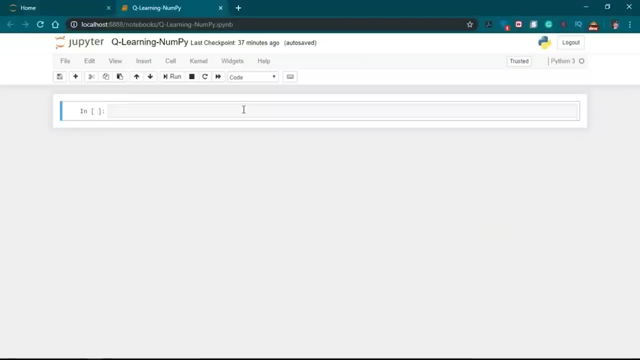 notebook and I'll name it as Q learning NumPy. Okay, so let's define the states, But before that, what we need to do is import NumPy, because we're going to use NumPy for this purpose, And let's initialize the parameters, that is, the gamma and alpha parameters. So gamma is 0.75,. 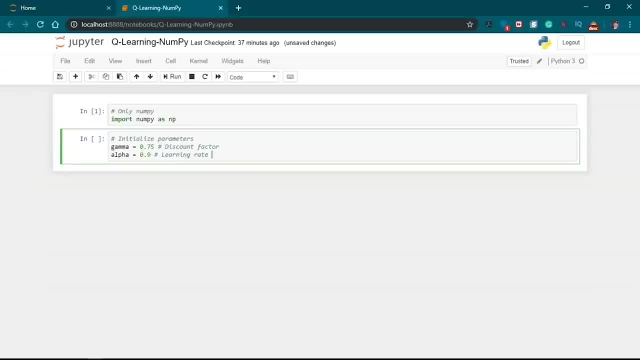 is the discount factor, whereas alpha is 0.9, which is the learning rate. now, next, what we're going to do is define the states and map it to numbers. so, as I mentioned earlier, l1 is 0 and till n line. we have defined the states in the 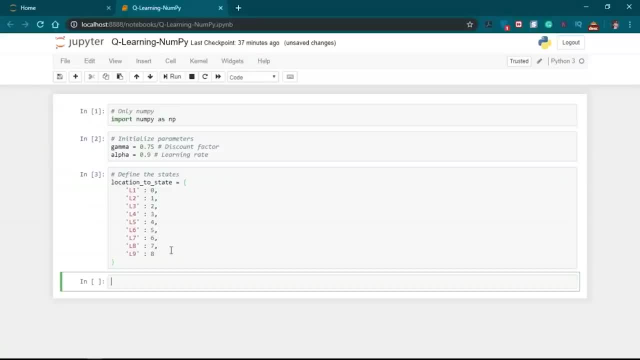 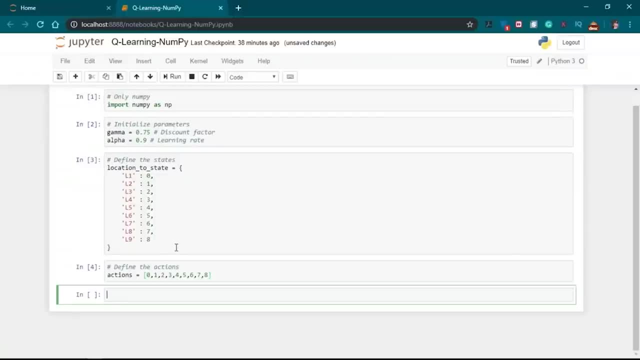 numerical form. now the next step is to define the actions, which is, as mentioned above, represent the transition to the next state. so, as you can see, here we have an array of actions from 0 to 8. now what we're going to do is define the. 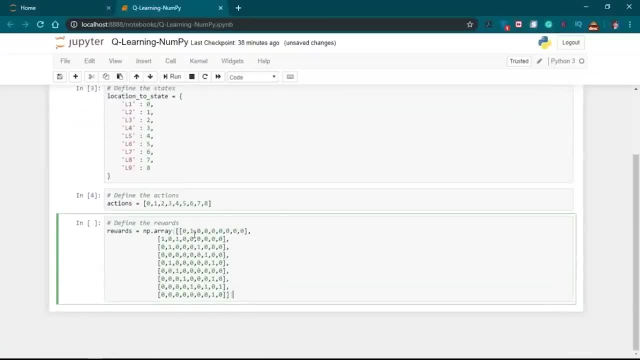 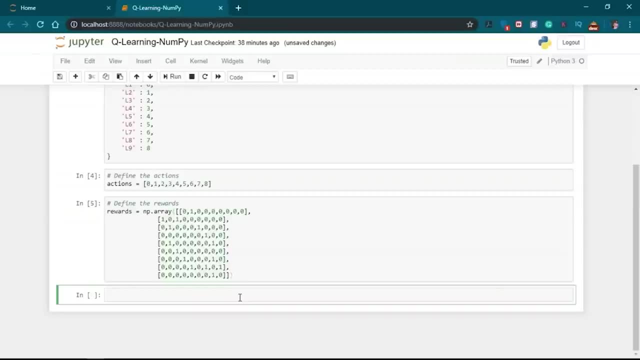 reward table. so, as you can see, it's the same matrix that we created just now, that I showed you just now. now, if you understood it correctly, there isn't any real barrier limitation as depicted in the image. for example, the transition l4 to l1 is allowed, but the reward will be 0 to. 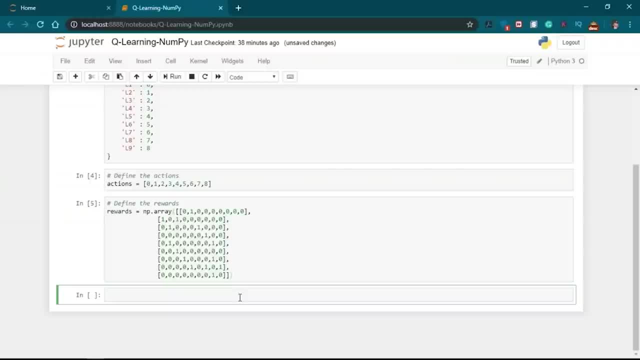 discourage that path or in tough situation, what we do is add a minus order on there so that it gets a negative reward. now in the above code snippet, as you can see here, we took each of the states and put once in the respective state that are directly reachable from the certain state. now, if we refer to 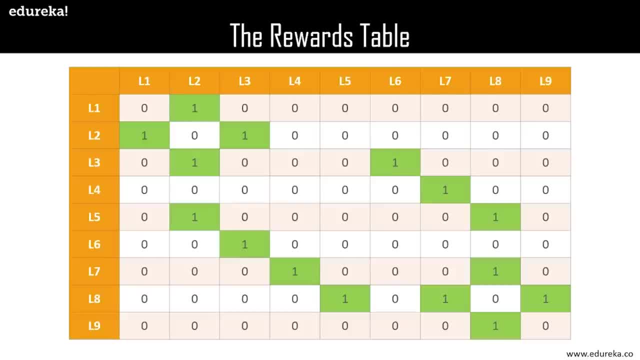 that reward table once again, what we created. the above array construction will be easy to understand. but one thing to note here is that we did not consider the top priority location l6 yet. we would also need an inverse mapping from the states back to its original state. 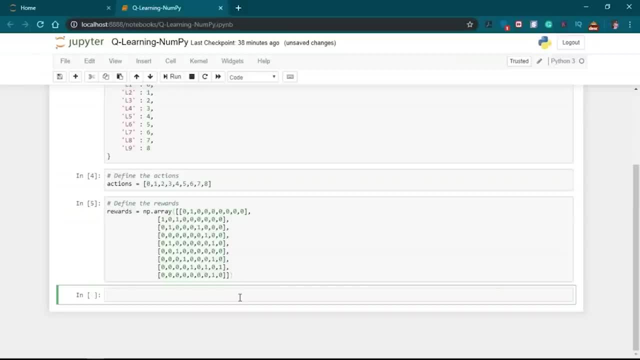 there isn't any real barrier limitation as depicted in the image. For example, the transition L4 to L1 is allowed, but the reward will be 0 to discourage that path Or in tough situation, what we do is add a minus on there so that it gets a negative. 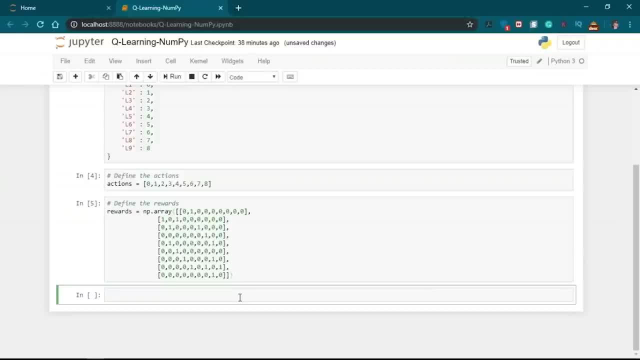 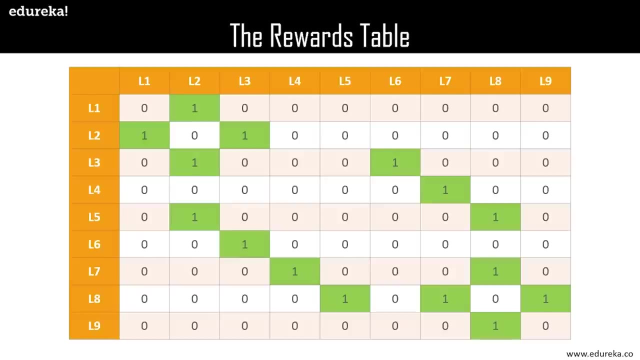 Now, in the above quote snippet, as you can see here, we took each of the states and put ones in the respective state that are directly reachable from the certain state. Now, if we refer to that reward table once again which we created, the above array construction will be easy to. 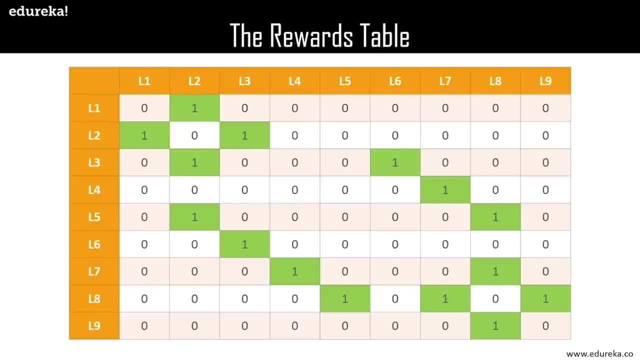 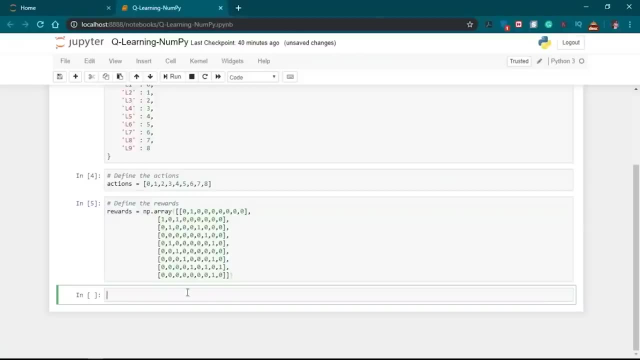 understand. But one thing to note here is that we did not consider the top priority location L6 yet. We would also need an inverse mapping from the states back to its original location, and it will be cleaner When we reach to the other depths of the algorithms. So for that, what we're going to do is have the inverse map, location state to location. 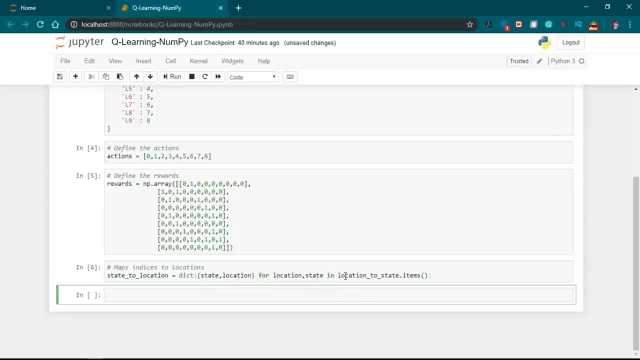 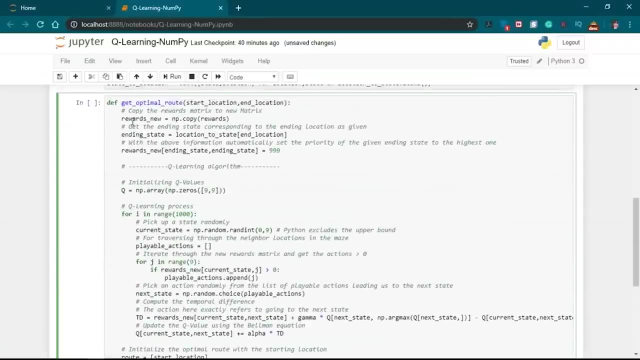 We will take the distinct state and location and convert it back. Now what we'll do is we'll now define a function, get optimal, which is the get optimal route, which will have a start location and an end location. Don't worry, the code is big, but I'll explain you each and every bit of the code. 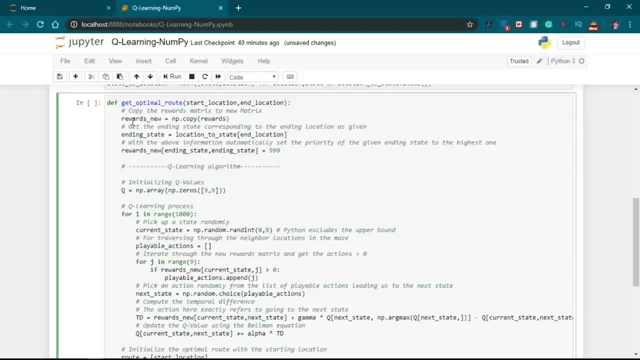 So now the get optimal route function will take two arguments- the starting location in the warehouse And the end location in the warehouse respectively- And it will return the optimal route for reaching the end location from the starting location in the form of an ordered list containing the letters. 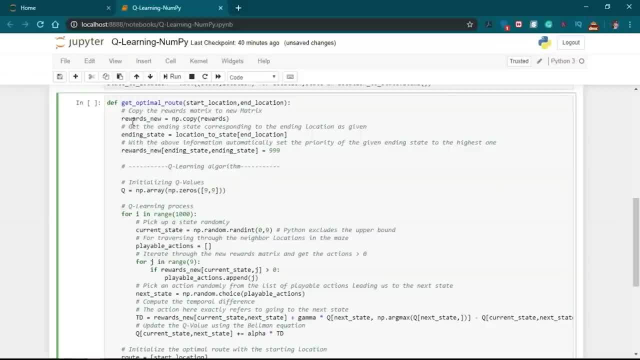 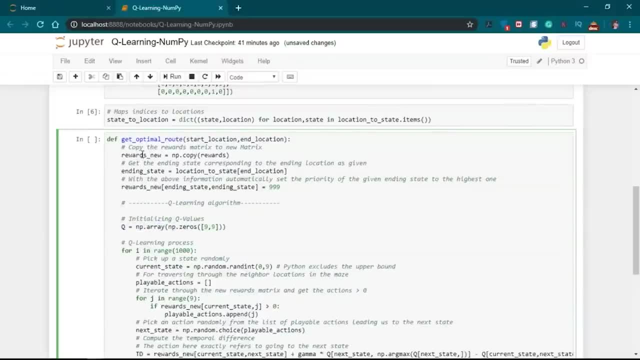 So we'll start by defining the function by initializing the Q values to be all 0s. So, as you can see here we have given the q values to be 0. But before that, what we need to do is copy the reward matrix to a new one. 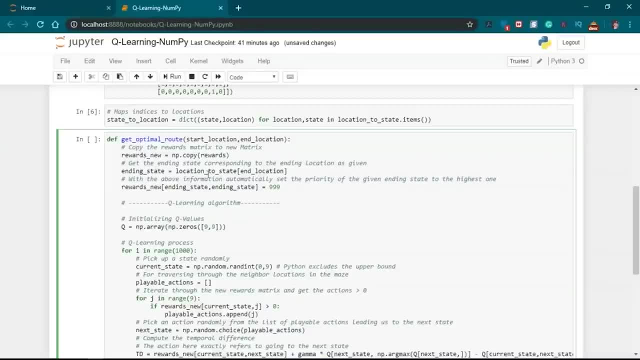 so this is the rewards, new. and next, again, what we're going to do is get the ending state corresponding to the ending location and with this information, automatically we'll set the priority of the given ending state to the highest one. that we are not defining it now, but we'll 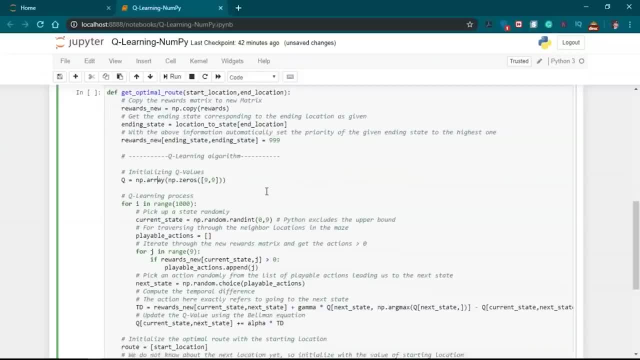 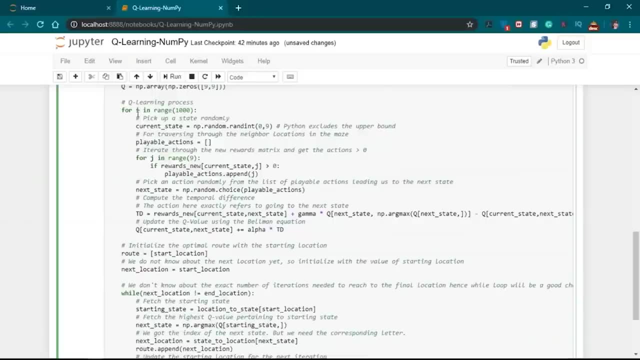 automatically set the priority of the given ending state as 999. so what we're going to do is initialize the q values to be 0 and in the q learning process, what you can see here, we are taking i in range 1000 and we're going to pick up a state randomly, so we're going to use the 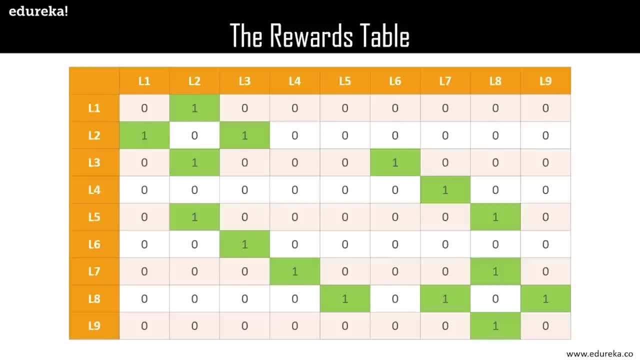 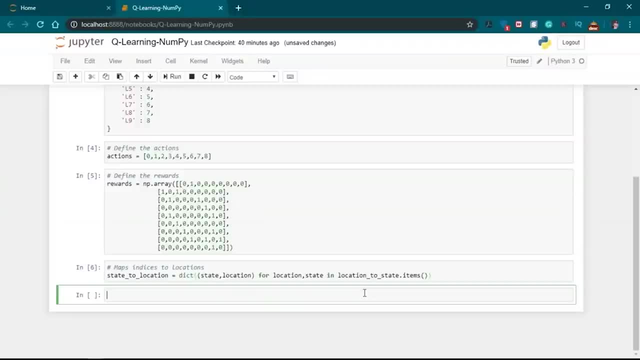 location, and it will be cleaner when we reach to the other depths of the algorithms. so for that, what we're going to do is have the inverse map, location, state to location. we will take the distinct state and location and convert it back. now what we'll do is we'll now define a function, get optimal- which is: 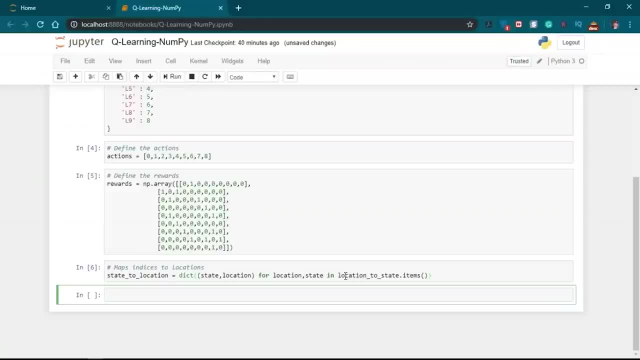 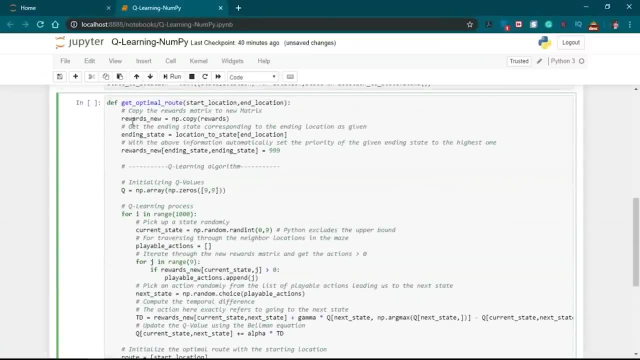 the get optimal route, which will have a start location and an end location. don't worry, the code is big, but I'll explain you how to do that in a minute in your each and every bit of the code. now the get optimal route function will take two arguments: the starting location in the warehouse and the end location in. 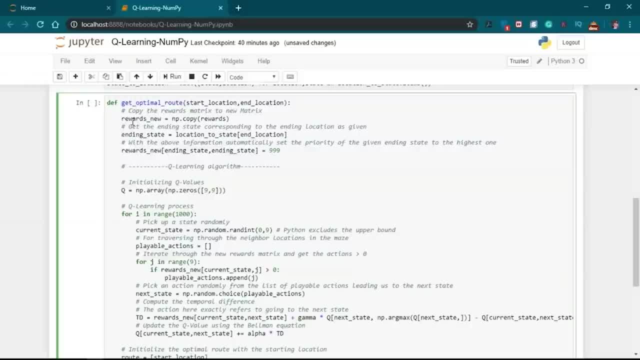 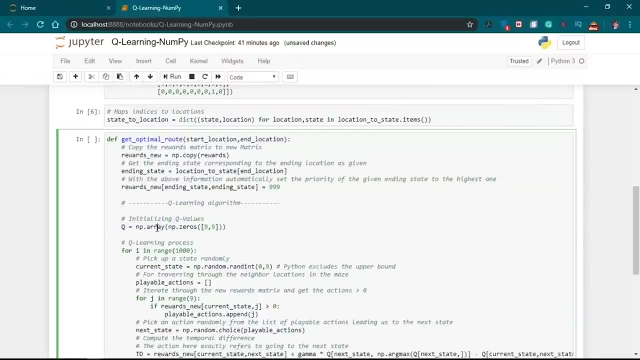 the warehouse respectively, and it will return the optimal route for reaching the end location from the starting location in the form of an ordered list containing the letters. so we'll start by defining the function by initializing the Q values to be all zeros. so, as you can see, here we have given the Q values. 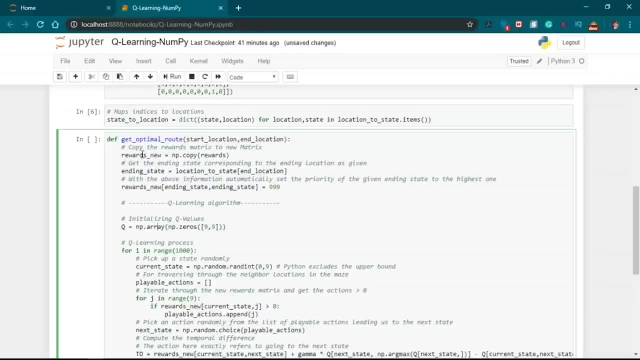 to be zero, but before that, what we need to do is copy the reward matrix to a new one. so this is the rewards, new and next again. what we're going to do is get the ending state corresponding to the ending location and with this information automatically will set the priority of. 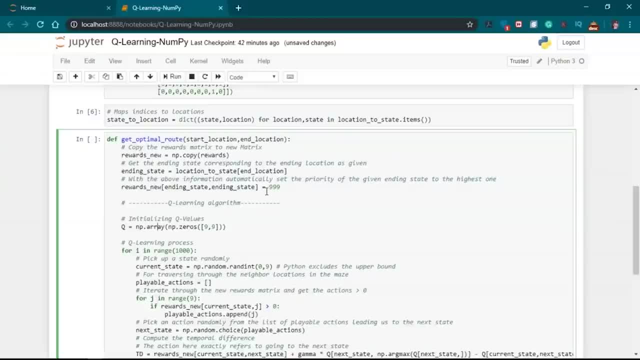 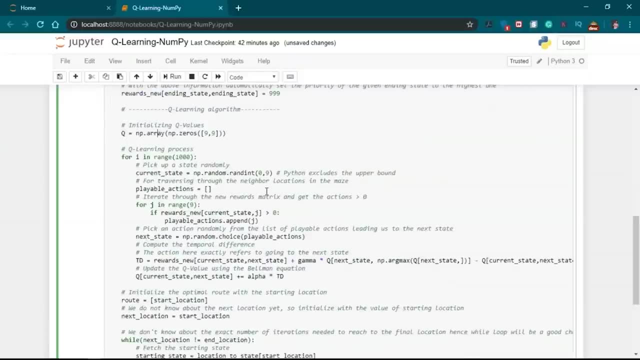 the given ending state to the highest one, that we are not defining it now, but will automatically set the priority of the given ending state as 999. so what we're going to do is initialize the Q values to be zero and in the Q learning process, what you can see here we are taking I in range. 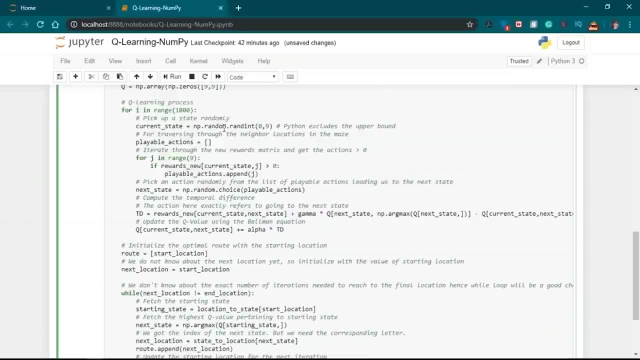 1000 and we're gonna pick up a state randomly. so we're gonna use the np dot random rant int and for traversing through the neighbor location in the same maze, we're gonna iterate to the new reward matrix and get the actions which are greater than zero, and after that what we're going to do is pick an action. 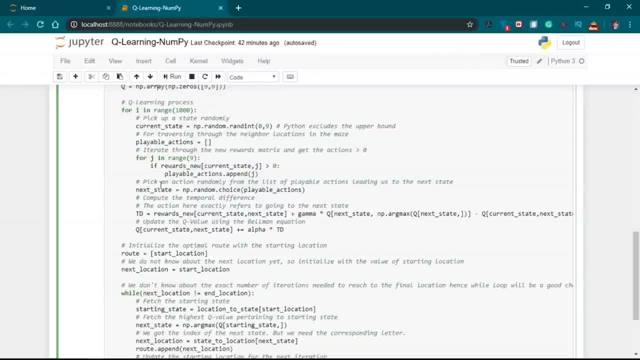 randomly from the list of the playable actions in years to the next state. we're gonna compute the temporal difference, which is TD, which is the rewards plus gamma, into the queue of next state and we'll take npargmax of q of next state minus q of the current state. we're going to then update. 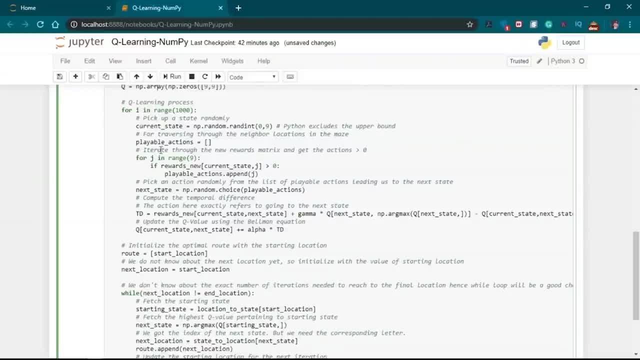 nprandom rand int. and for traversing through the neighbor location in the same maze. we're going to iterate through the new reward matrix and get the actions which are greater than 0, and after that what we're going to do is pick an action randomly from the list of the playable actions in years to. 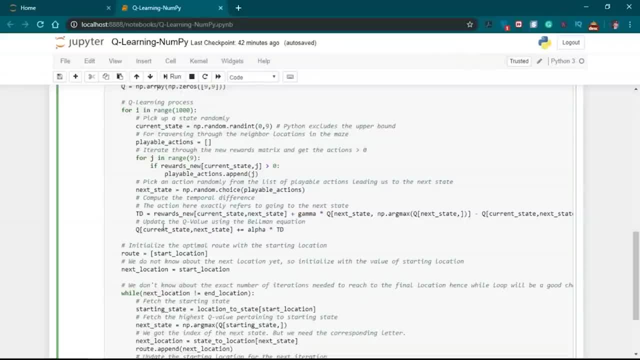 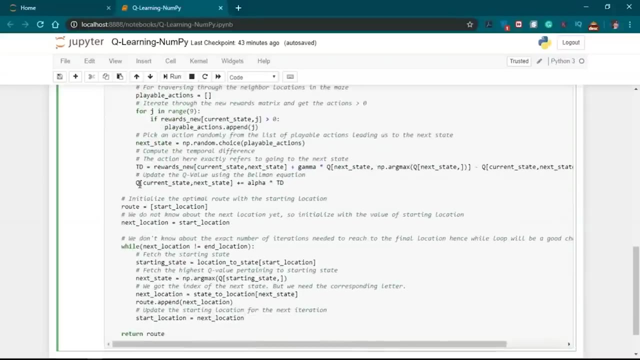 the next state. we're going to compute the temporal difference, which is td, which is the rewards plus gamma, into the q of next state and we'll take npargmax of q of next state minus q of the current state. we're going to then update the q values using the bellman equation. as you can see, here we have the. 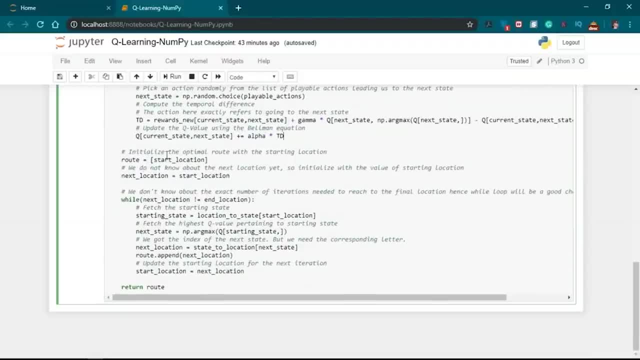 bellman equation and we're going to update the q values and after that we're going to initialize the optimal route with the starting location. now here we do not know what the next location yet, so initialize it with the value of the starting location, which again is the random location. 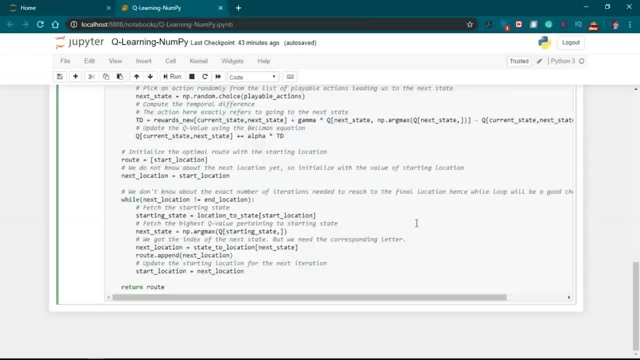 now we do not know what the exact number of iterations needed to reach to the final location. hence, while low will be a good choice for the iteration. so we're going to fetch the starting state, fetch the highest q value penetrating to the starting state, we go to the index of the next state. 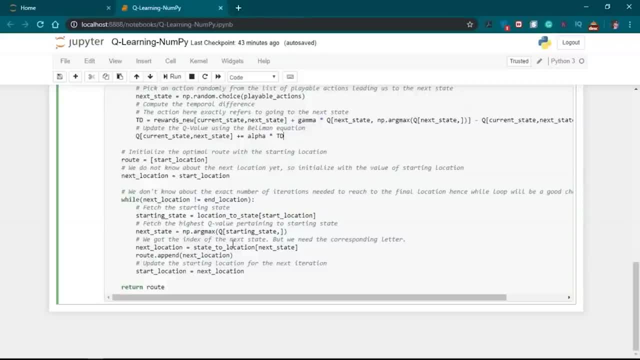 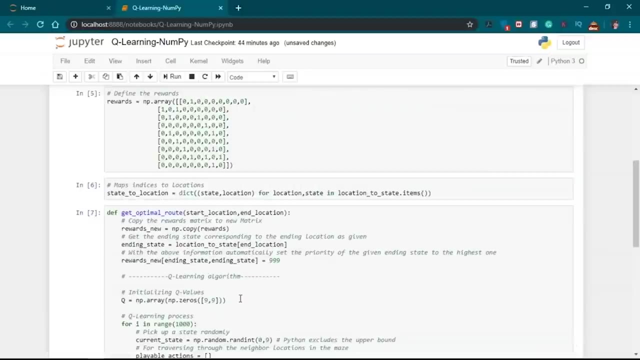 but we need the corresponding letter. so we're going to use that state to location function we just mentioned there, and after that we're going to update the starting location, for the next iteration will return the root, so let's take the starting location of l9 and the end location of l1 and see. 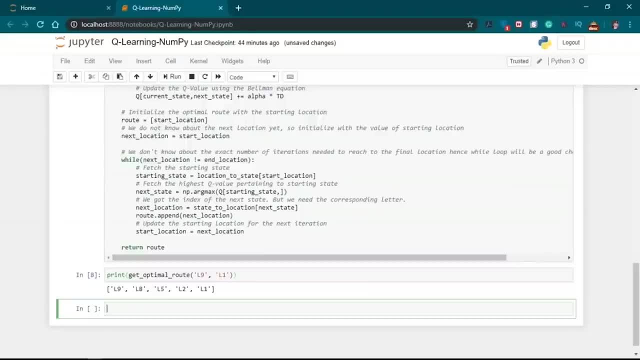 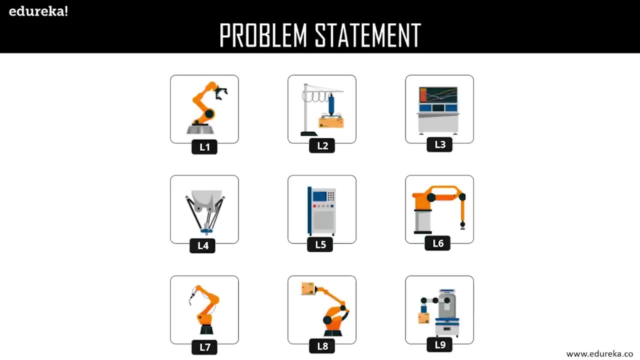 what part do we actually get? so, as you can see, here we get l9, l8, l5, l2 and l1 and if you have a look at the image here we have, if we start from l9 to l1, we got l8, l5, l2, l1, l8, l5, l2, l1. that would 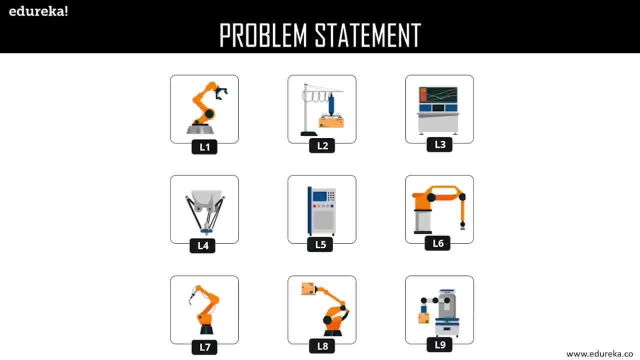 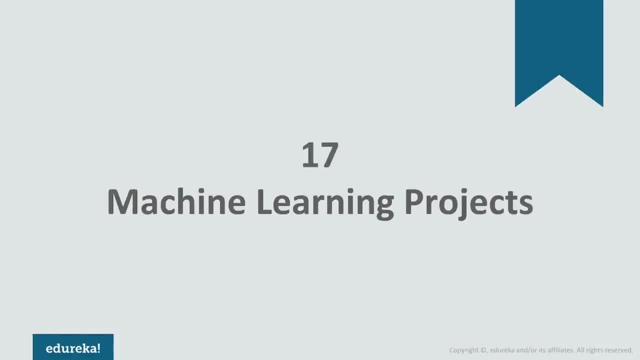 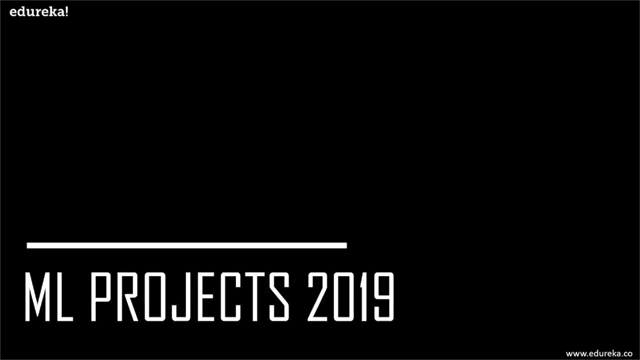 yield us the maximum value or the maximum reward for the robot. so now we have come to the end of this Q learning session. the past year has seen a lot of great examples for machine learning, and many new high-impact application of machine learning were discovered and brought to light. 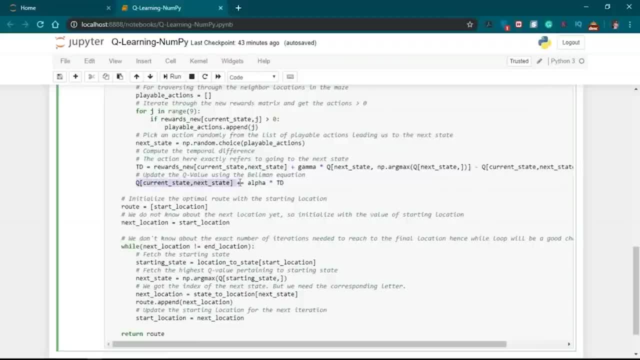 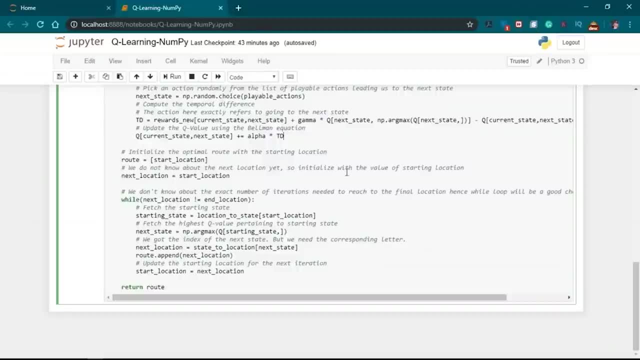 the q values using the bellman equation. as you can see, here we have the bellman equation and we're going to update the q values and after that we're going to initialize the optimal route with the starting location. now here we do not know what the next location yet, so initialize it with the. 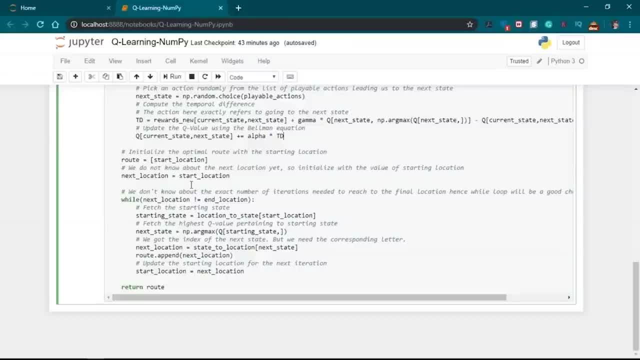 value of the starting location, which again is the random location. now we do not know what the exact number of iterations needed to reach to the final location. hence, while low, will be a good choice for the iteration. so we're going to fetch the starting state, fetch the highest q value. 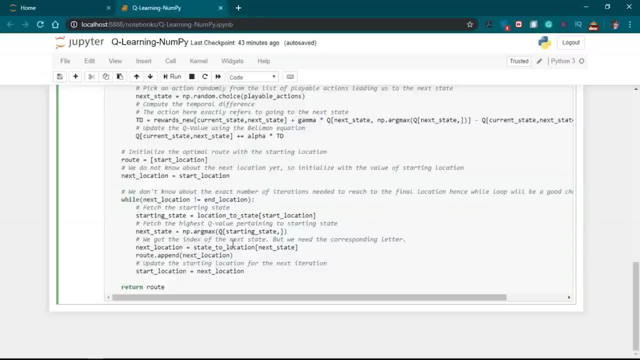 penetrating to the starting state, we go to the index of the next state, but we need the corresponding letter. so we're going to use that state to location function we just mentioned there and after that we're going to update the starting location for the next iteration and finally, we'll return the 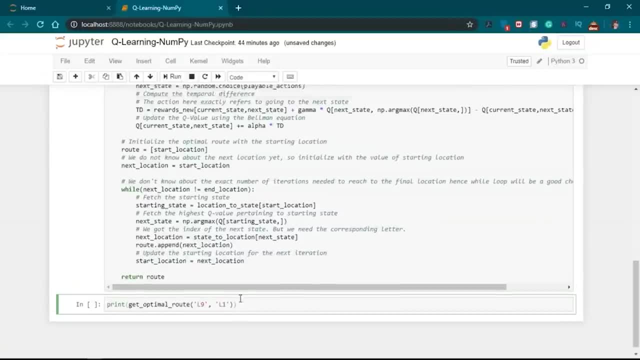 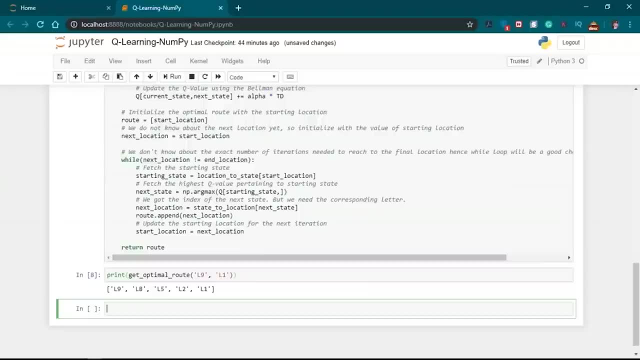 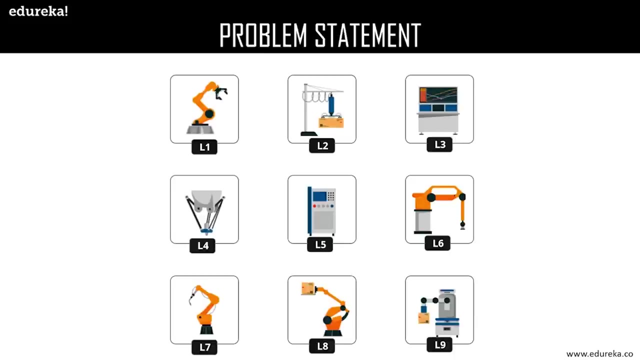 route. so let's take the starting location of l9 and the end location of l1 and see what part do we actually get. so, as you can see here, we get l9, l8, l5, l2 and l1, and if you have a look at the image, 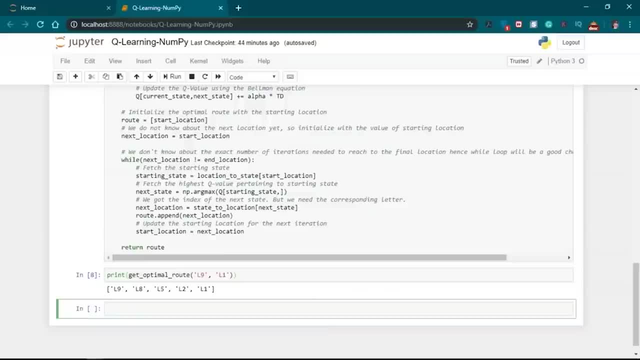 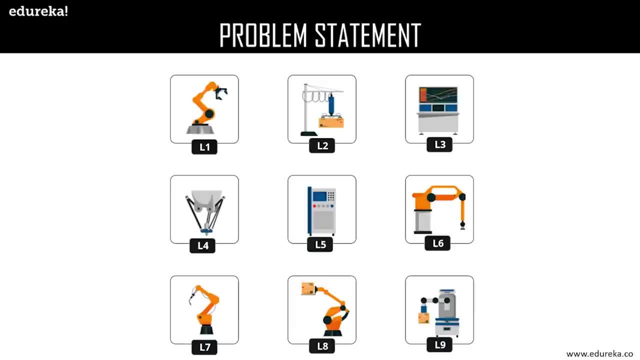 here we have. if we start from l9 to l1, we got l8, l5, l2, l1, l8, l5, l2, l1. that would yield us the maximum value or the maximum reward for the next iteration. so let's take the starting location of l9 and the 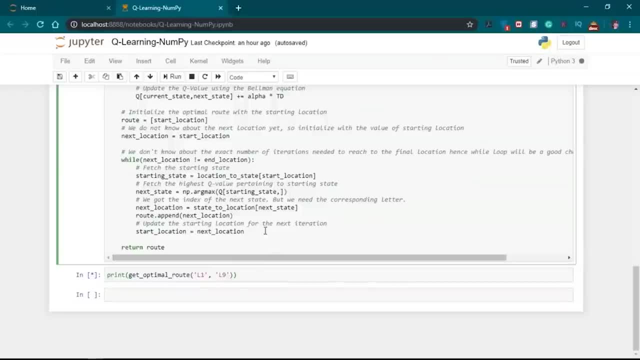 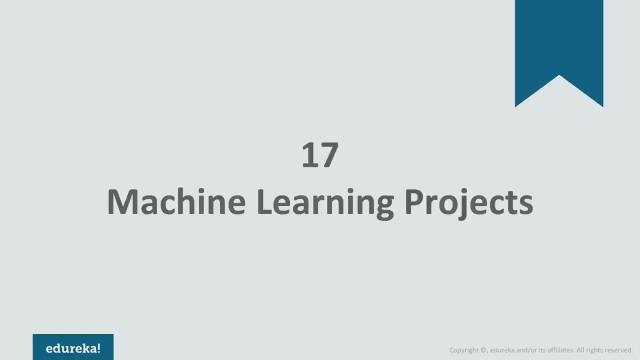 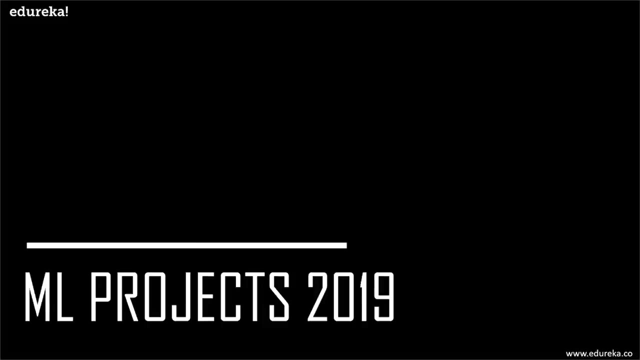 end location of the robot. so now we have come to the end of this q learning session. so, and so we have come to the end of this Q learning session. the very first step in this task was to figure out the five key features that we needed to 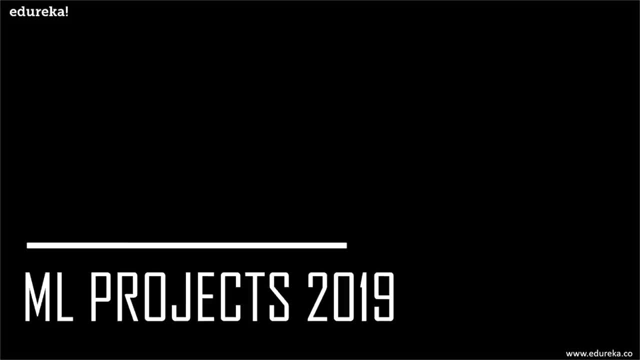 What was the first step in operating the robot? How did we develop the first step in operating the robot? So now we have come to the end of this. Q learning session was easily the most talked about domain within the community with the likes of ulm, fit and, but being open sourced. so let's have a look at some of the amazing. 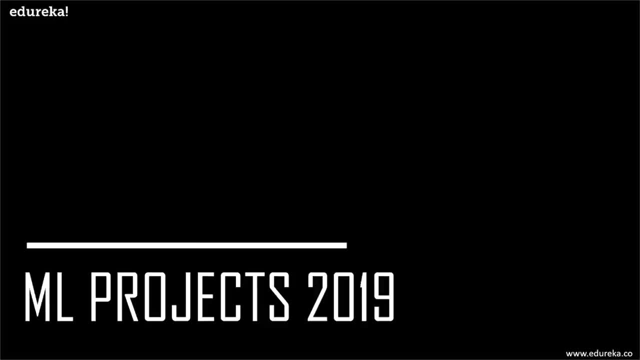 especially in the healthcare finance, the speech recognition, augmented reality and much more complex tools, 3d and video applications. now, natural language processing was easily the most talked about domain within the community, with the likes of ulmf, it, and, but being open sourced, so let's have a look. 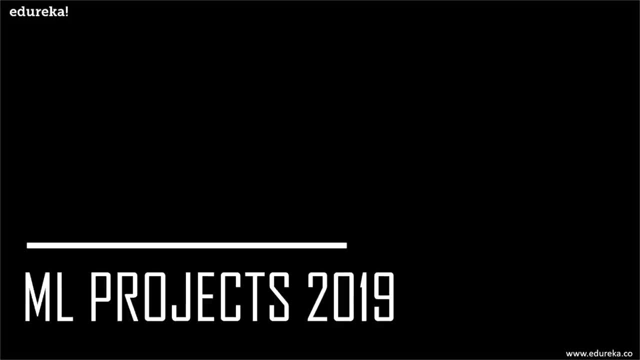 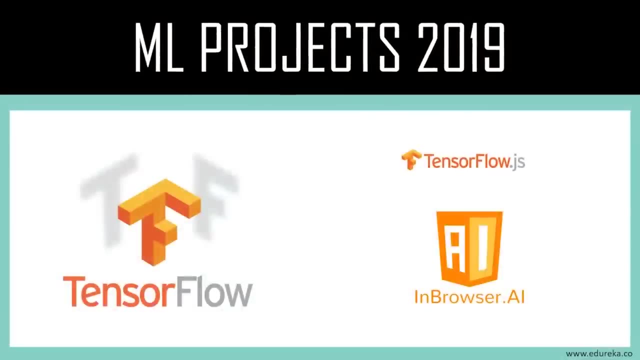 at some of the amazing machine learning projects which are open sourced. the code is available for you and those were discussed in this 2018 to 19 spectrum. so the first and the foremost is tensorflowjs. now machine learning in the browser affects the. a few years back and a stunning reality. now a lot of us in this field are welded to our favorite. 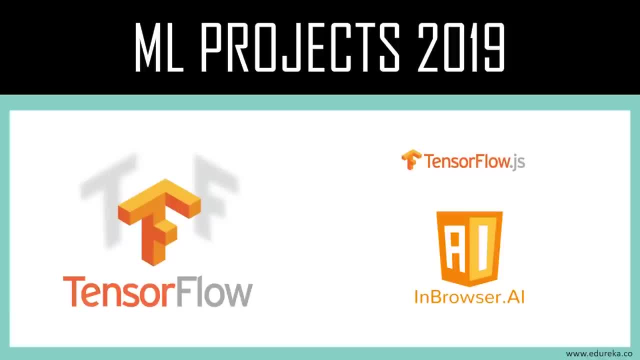 ides, but tensorflowjs has the potential to change your habits. it's become a very popular release since its release earlier this year and continues to amaze with its flexibility now, as the repository states. there are primarily three major features of tensorflowjs: develop, machine learning and 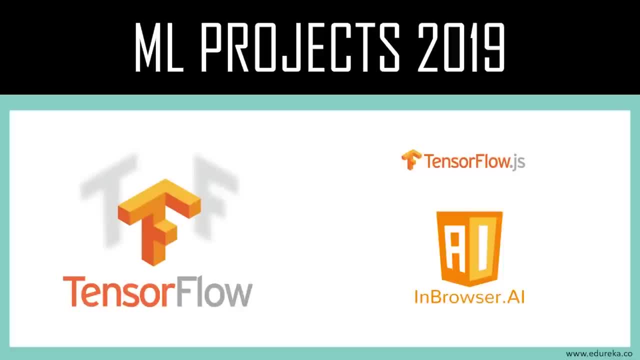 deep learning models in your browser itself. run pre-excessing tensorflow models within the browser. we train our fighting these pred retirals as well, and if you are familiar with Keras, the high level layers API, will seem quite familiar, but there are plenty of examples available. 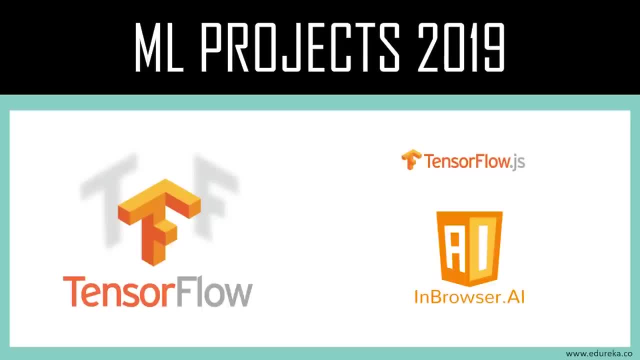 on kit of repository. so do check out those clicks to quick in your learning code and, as i mentioned earlier, i'll leave the links to all of these open source machine learning projects in the description below. next, what we will discuss is detectron. it is developed by Facebook and made 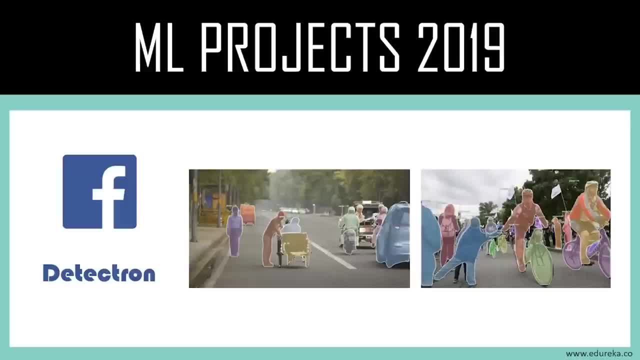 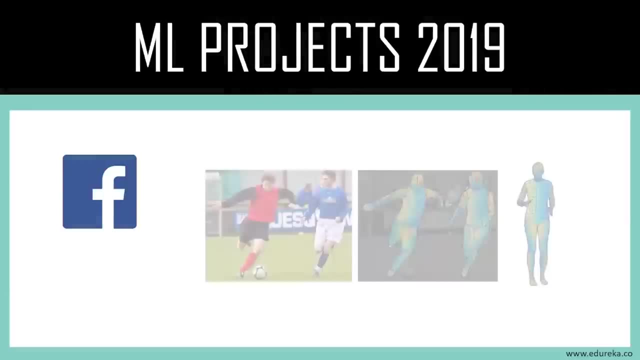 a huge splash went into, was earlier launched in 2018. it was developed by facebook's ai research team, which is fair, and it implements the state-of-the-art object detection frameworks. it is written in python and has helped enable multiple projects, including the dense force. now we'll know what exactly is. 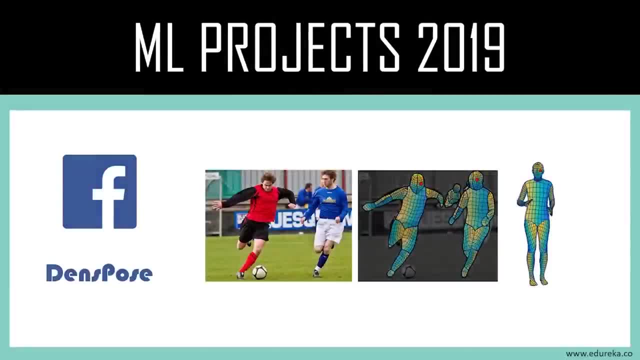 dense force after this example. and this repository contains the code of over 70 pre-trained models, so it's a very good open source model, guys, so do check it out now. the moment i talked about dense force, that's the next one i'm going to talk about. so dense force is dense human pose estimation in. 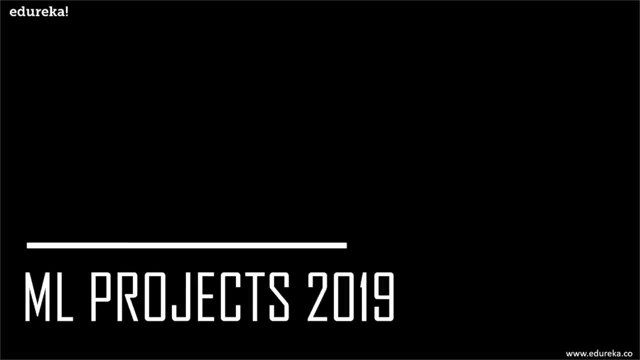 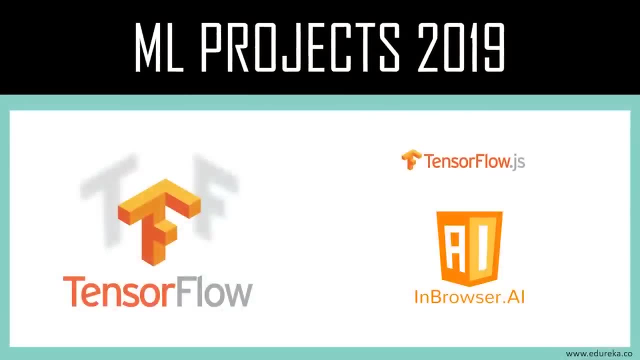 machine learning projects which are open sourced, the code is available for you, and those were discussed in this 2018 to 19 spectrum. so the first and the foremost is tensorflowjs. now machine learning in the browser: a fictional thought a few years back and a stunning reality now. a lot of us in this field are welded to 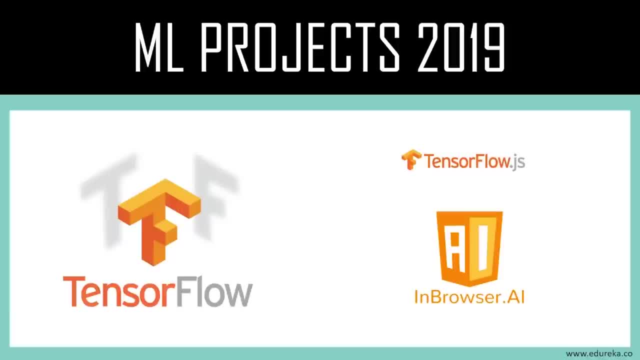 our favorite IDEs, but tensorflowjs has the potential to change your habits. it's become a very popular release since its release earlier this year and continues to amaze with its flexibility. now, as the repository states. there are primarily three major features of tensorflowjs: develop machine. 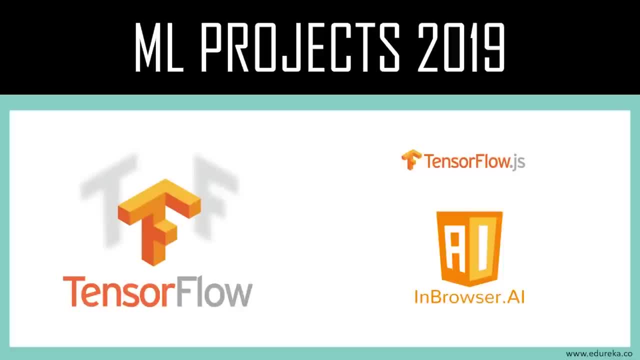 learning and deep learning models in your browser itself run pre accessing tensorflow models within the browser. read train are finding these prediction models as well, and if you are familiar with Keras, the high-level layers API, will seem quite familiar. but there are plenty of examples available on GitHub repository, so do check out those clicks. 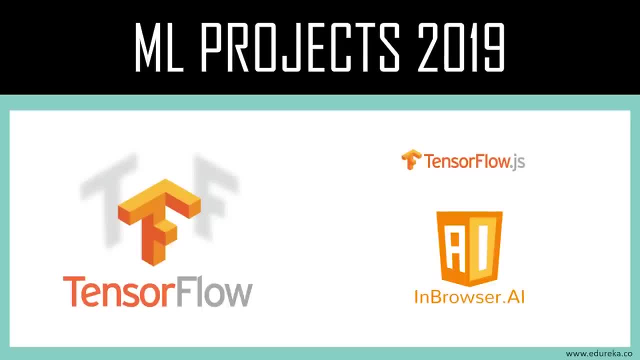 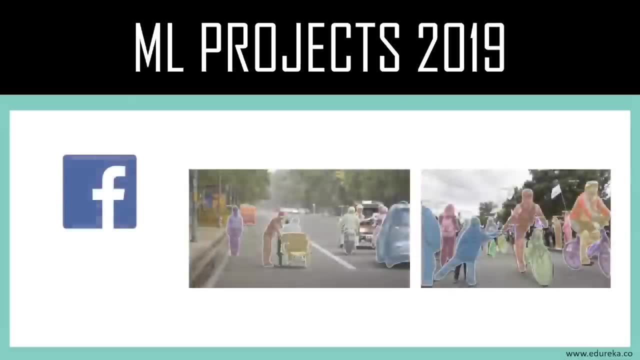 to quicken your learning curve and, as I mentioned earlier, I'll leave the links to all of these open source machine learning projects in the description below the next what we're going to discuss is Detectron. it is developed by Facebook and made a huge splash when it was earlier launched. 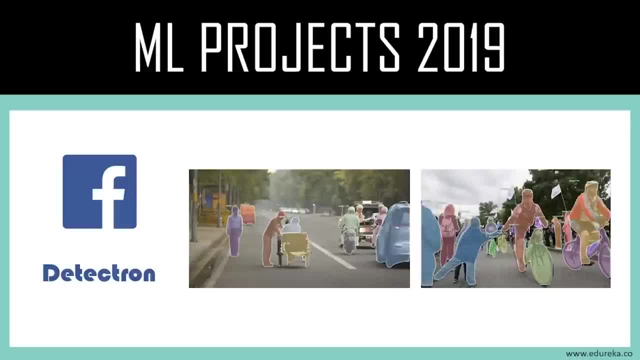 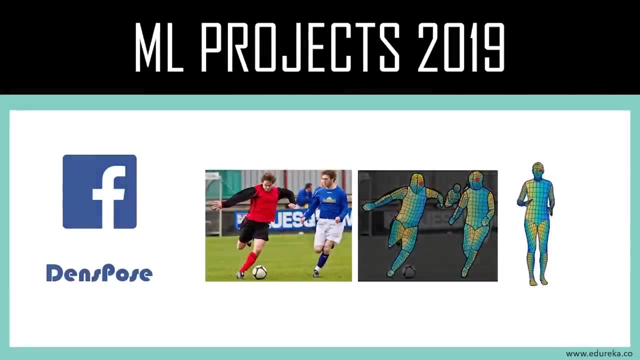 in 2018. it was developed by Facebook's AI research team, which is FAIR, and it implements the state-of-the-art object detection frameworks. it is written in Python and has helped enable multiple projects, including the dense force. now we'll know what exactly is dense force after this example and this repository. 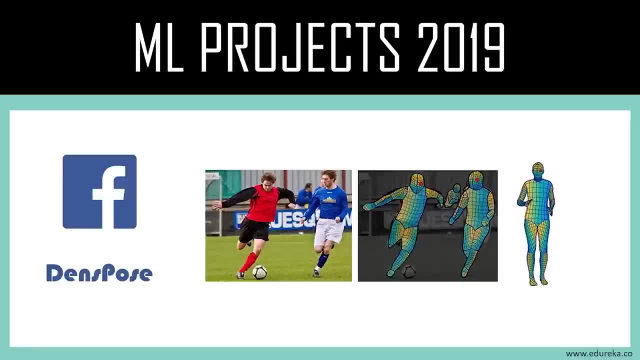 contains the code of over 70 pre-trained models, so it's a very good open source model, guys, so do check it out now. the moment I talked about dense force- that's the next one I'm going to talk about- is the open source model, which is a very good open source model, guys, so do check it out now. the moment I talked about dense force, that's the next one I'm going to talk about. 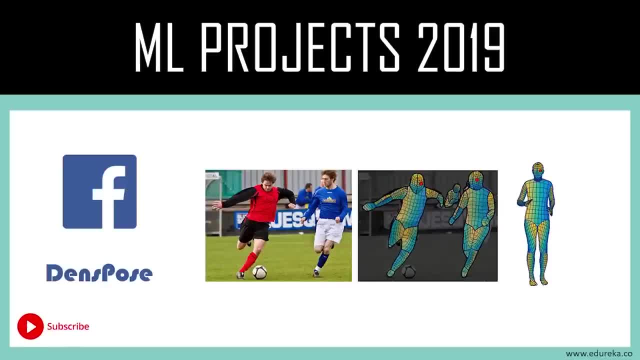 about. so dense force is dense human force estimation in the wild. now the code to train and evaluate your own dense force using the RCNN model is included here and I've given the link to the open source code in the description below, and there are notebooks available as well to visualize the dense force coco data set. 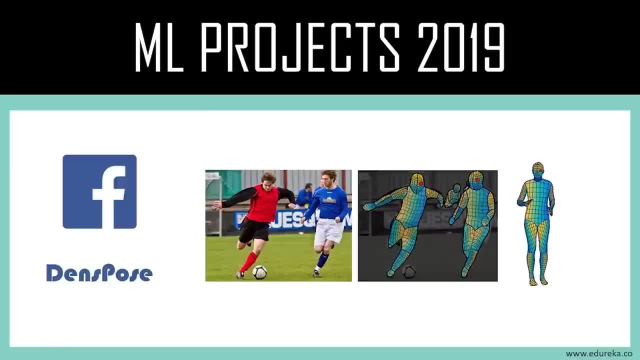 the wild now. the code to train and evaluate your own dense force using the rcnn model is included here, and i've given the link to the open source code in the description below, and there are notebooks available as well to visualize the dense force coco data set now. next in our list. we have 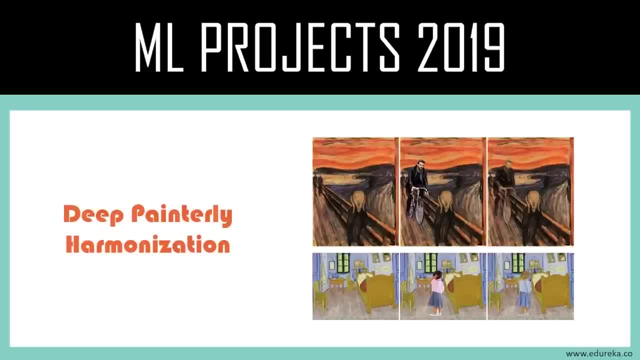 deep painterly harmonization. now i want you to take a moment to just admire the above images. can you tell which ones were done by a human and which one by a machine? i certainly could not. now here, the first frame is the input image, the original one, and the third frame, as you can see here, has been generated by this technique. amazing. 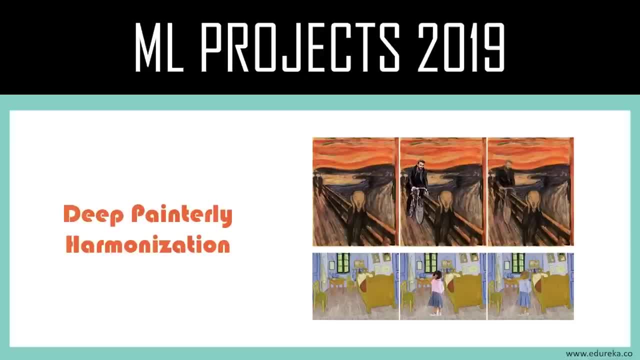 right. the algorithm adds an external object to your choosing to any image and manages it to make it look like nothing touched it. now make sure you check out the code and try to implement it on different sets of images yourself. it is really, really fun. but talking about images, we have image. 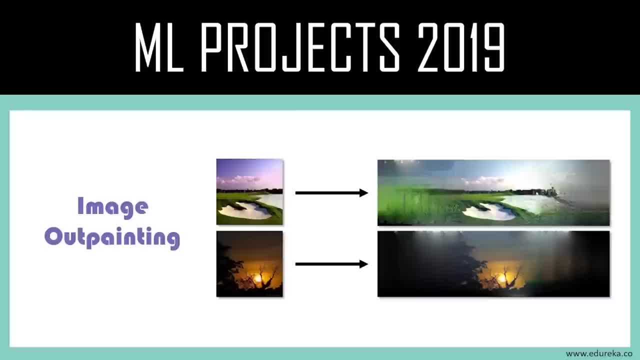 outpainting. now what if i give you an image and ask you to extend its boundaries by imagining what it would look like when the entire scene was captured? you would understandably turn to some image editing software. but here's the awesome news: you can achieve it in few lines of code. 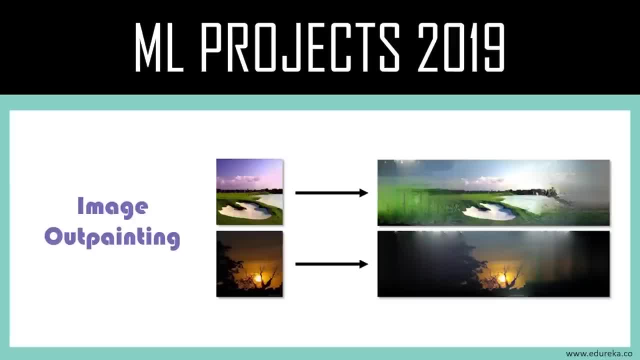 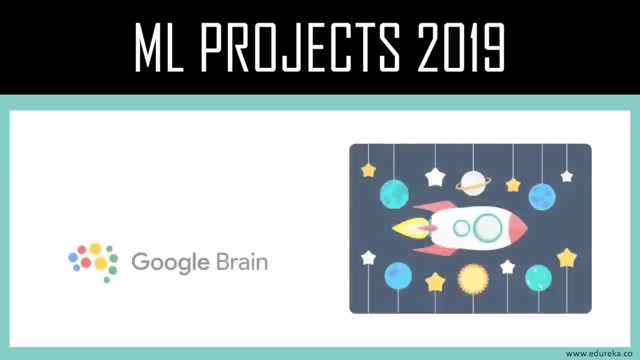 which is the image outpainting. now, this project is a keras implementation of stanford image outpainting paper, which is incredibly cool and illustrated paper, and this is how most research papers should be. do check it out, guys, and see how you can implement it. now let's talk about audio processing, which is 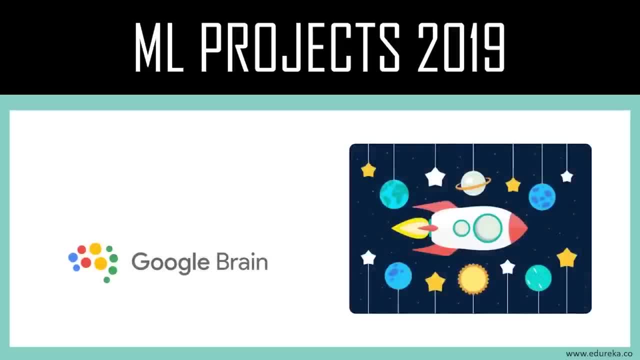 an another field where machine learning has started to make it smart. it is not just limited to generic music. you can do tasks like audio classification, fingerprinting, segmentation, tagging and much more, and there is a lot that's still yet to be explored. and, who knows, perhaps you could use this project to pioneer your way to the top. now what if you want to discover? 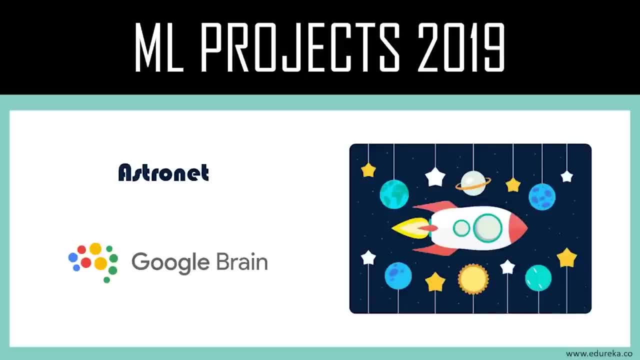 your own planner. now, that might perhaps be overstating things a bit, but the astronet repository will definitely get you close. the google brain team discovered two new planets in december 2017 by applying the astronet. it's a deep neural network meant for working with. 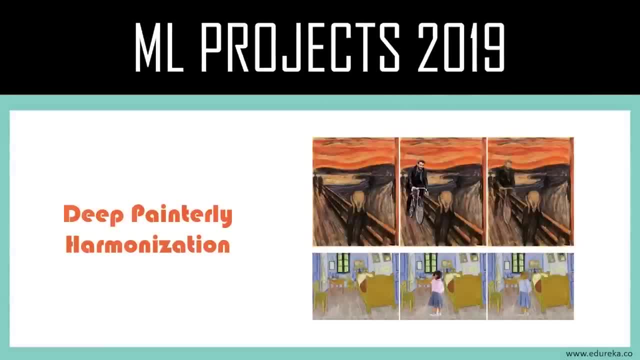 now next in our list, we have deep painterly harmonization. now I want you to take a moment to just admire the above images. can you tell which ones were done by a human and which one by a machine? I certainly could not now here. the first frame is the input image, the 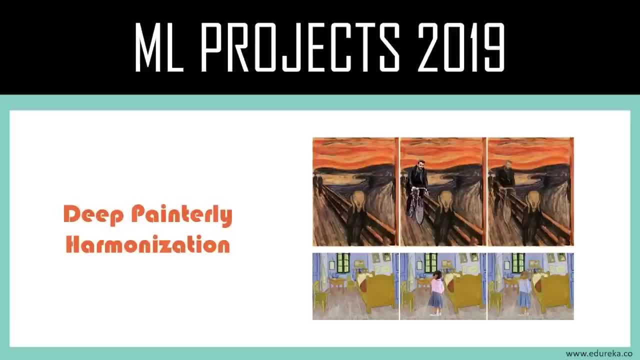 original one, and a third frame, as you can see here, has been generated by this technique. amazing, right. the algorithm adds an external object to your choosing to any image and manages it to make it look like nothing touched it. now make sure you check out the code and try to implement it on different sets of images. 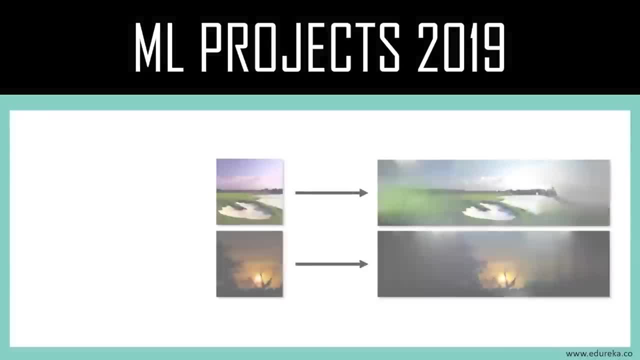 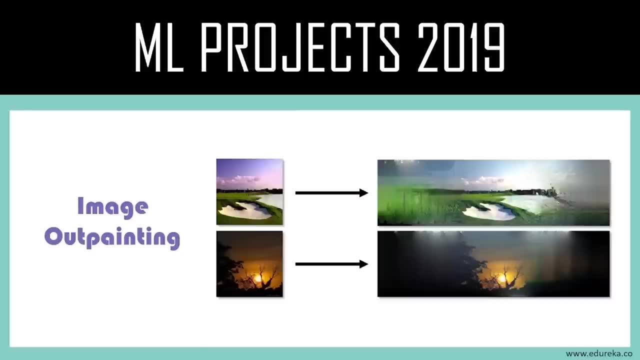 yourself. it is really, really fun. but talking about images, we have image out painting. now what if I give you an image and I ask you to extend its boundaries by imagining what it would look like when the entire scene was captured? you would understandably turn to some image. 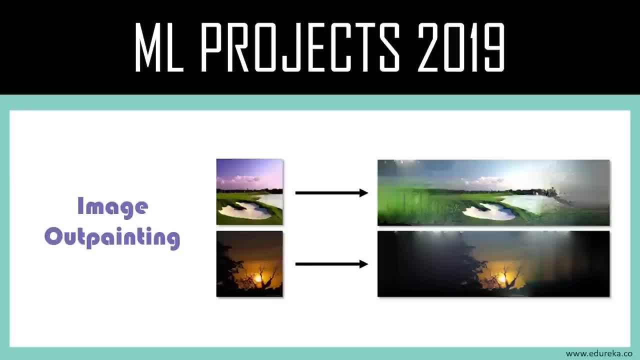 editing software. but here's the awesome news: you can achieve it in few lines of code, which is the image outpainting. now, this project is a Keras implementation of Stanford image outpainting paper, which is incredibly cool and illustrated paper, and this is how most research paper should be. I have given 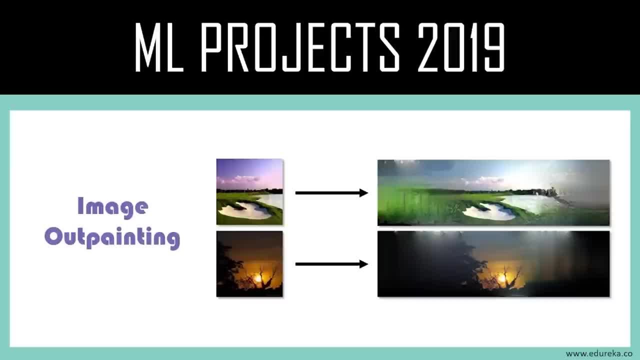 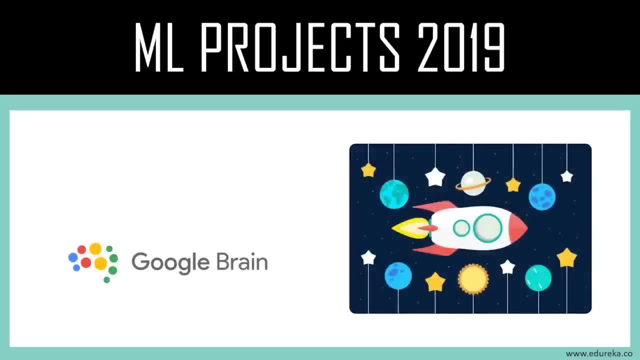 the links in the description below. do check it out, guys, and see how you can implement it. now let's talk about audio processing, which is an another field where machine learning has started to make it smart. it is not just limited to generate music. you can do tasks like audio. 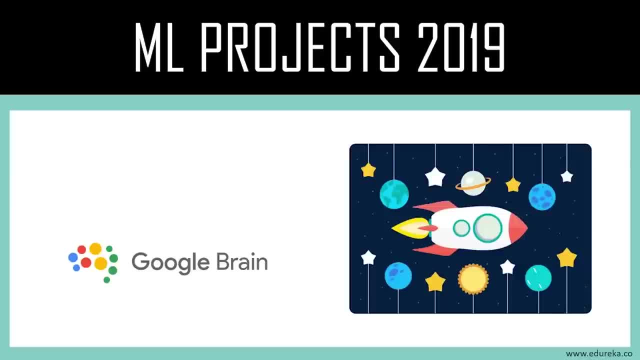 classification, fingerprinting, segmentation, tagging and much more, and there is a lot that's still yet to be explored. and, who knows, perhaps you could use this project to pioneer your way to the top. now what if you want to discover your own planner? now, that might perhaps be overstating things a bit, but the 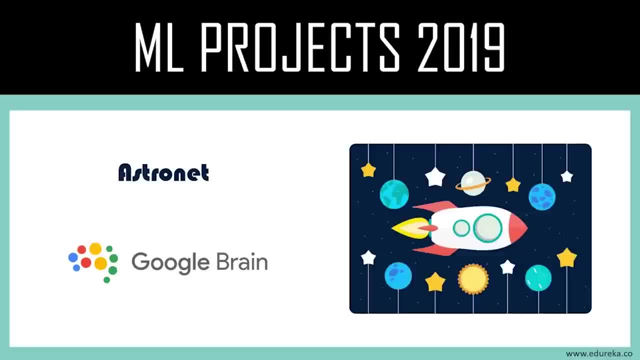 astronet repository will definitely be available in the future. if you want to get you close, the Google brain team discovered two new planets in December 2017 by applying the astronet. it's a deep neural network meant for working with astronomical data. it goes to show the far-ranging application of machine. 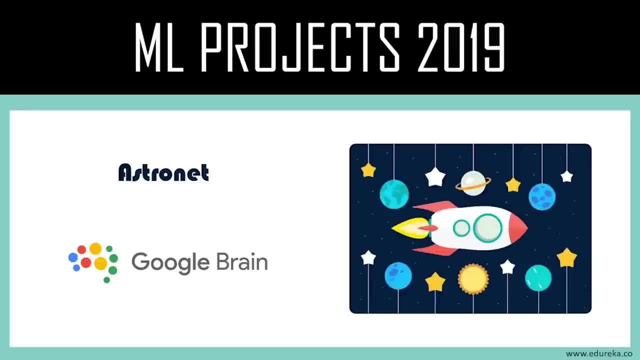 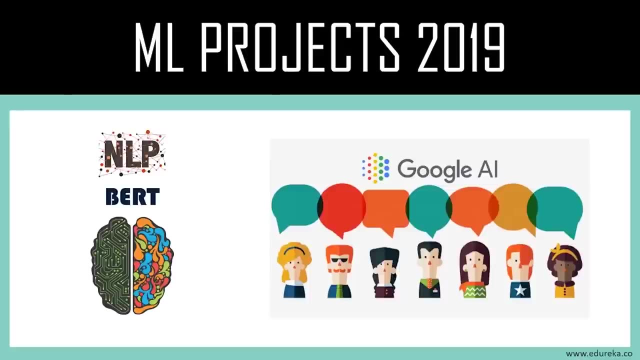 learning and was a truly monumental development. and now the team behind the technology has open-sourced the entire code. so go ahead and check out your own planet and, who knows, you might even have a planet on your name. now I could not possibly let this section pass by without mentioning the BRT, the Google, 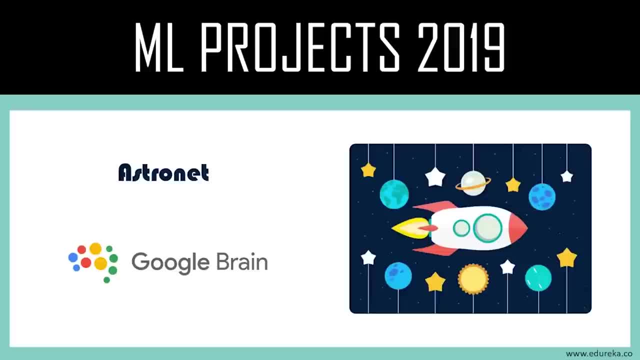 astronomical data. it goes to show the far-ranging application of machine learning and was a truly monumental development. and now the team behind the technology has open sourced the entire code. so go ahead and check out your own planet, and, who knows, you might even have a planet on your name. 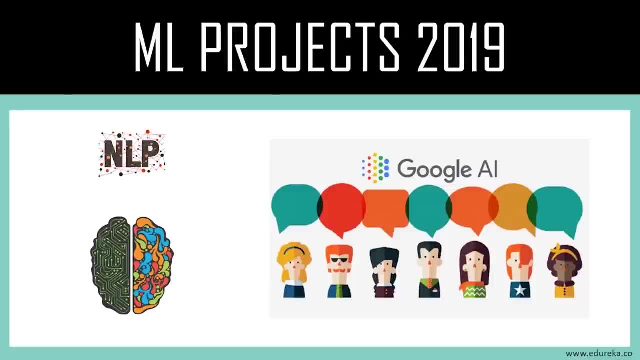 i could not possibly let this section pass by without mentioning the bert. the google ai's release has smashed record on its way to winning the hearts of nlp enthusiasts and experts alike. following ul mfit and elmo bert really blew away the competition with its performance. 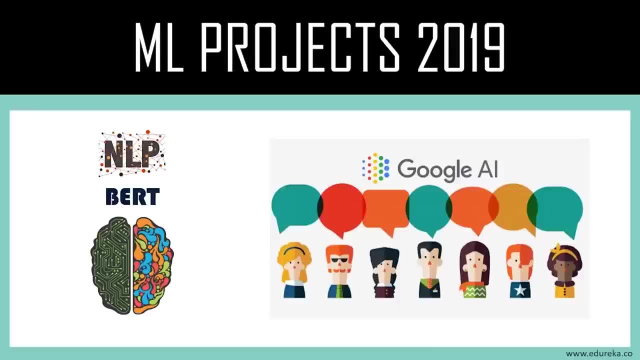 it obtained the state of art result on 11 nlp tasks. apart from the official google repository, there is a pytorch implementation of bird which is worth checking out. whether it makes an new era or not in natural language processing we will soon find out. now, aranet, i'm sure you guys 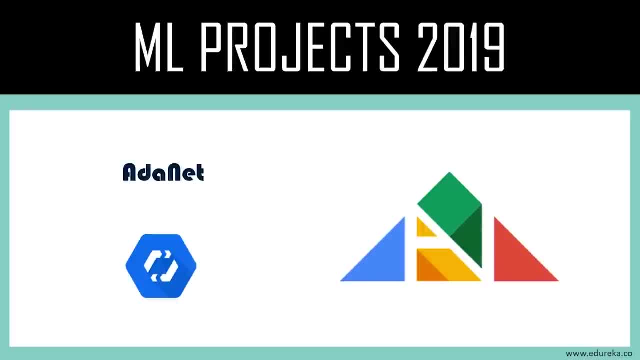 might have heard of it. it is a framework for automatically learning high quality models without requiring programming expertise, since it's a google invention. the framework is based on tensorflow and you can build ncable models using aranet and even extend it to use to train a neural network. 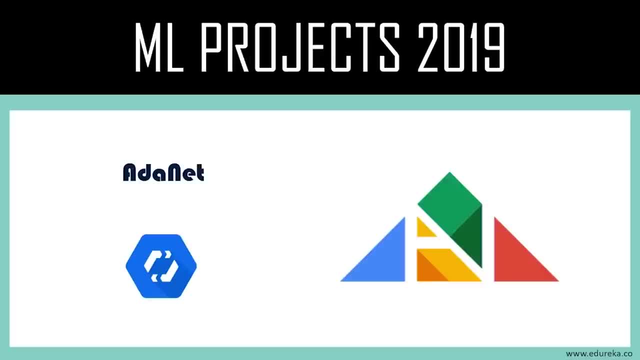 now. the github page contains the code, an example, the api documentation and other things to get your hands dirty. now trust me, if you are interested in learning more about nlp, you should definitely follow me. auto ml is the next big thing in our field now. if you follow a few researchers on. 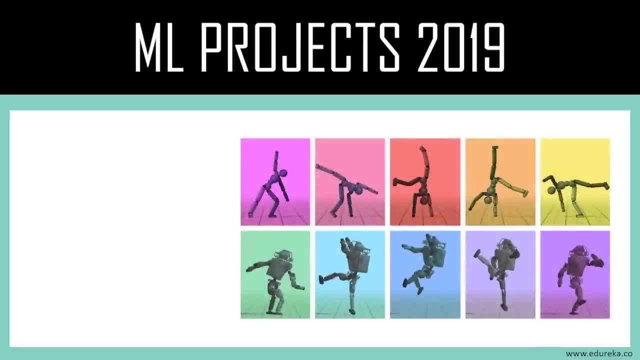 social media, you must have come across some of the images i am showing here in a video form: a stick, human running across the terrain or trying to stand up or some sort. now that my friends is reinforcement learning in action. now here's a signature example of it. 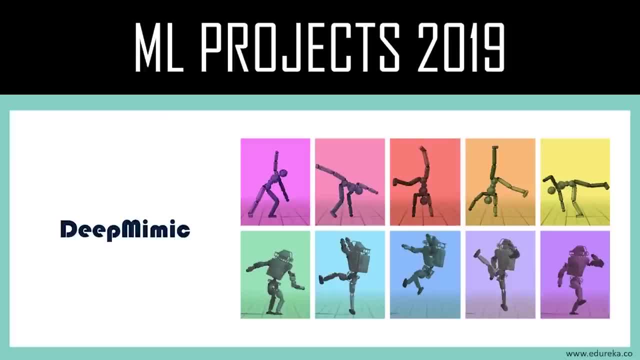 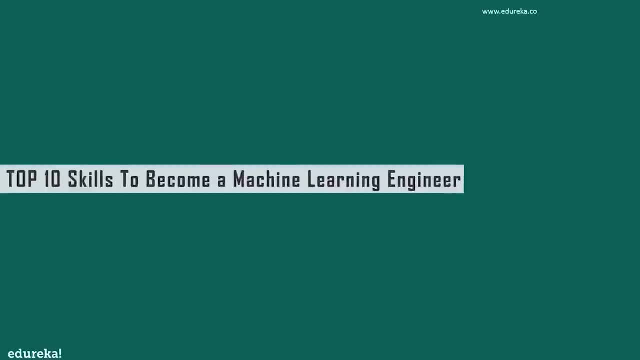 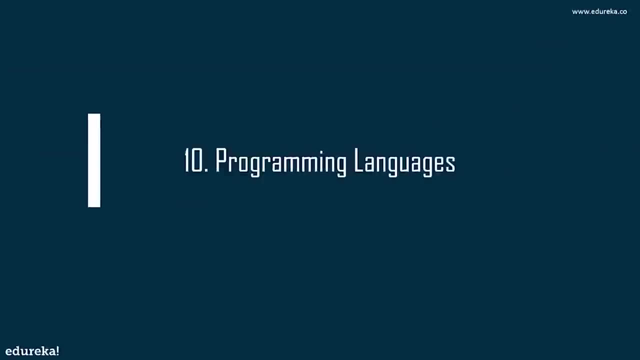 a framework to train a simulated humanoid to imitate multiple motion skill. so let's have a look at the top 10 skills which are required to become a successful machine learning engineer. so, starting with programming languages, python is the lingua franca of machine learning. you may have had exposure to python even if you weren't previously in programming. 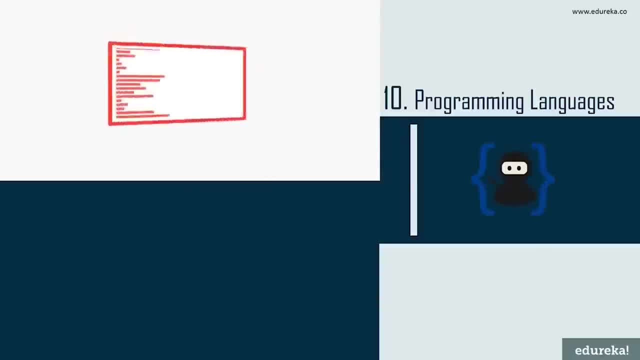 or in a computer science related field. however, it is important to have a solid understanding of classes and data structures. sometimes python won't be enough. often you'll encounter projects that need to leverage hardware for speed improvements. now make sure you're familiar with the basic algorithms, as well as the classes, memory, management and linking. now, if you want a job in. 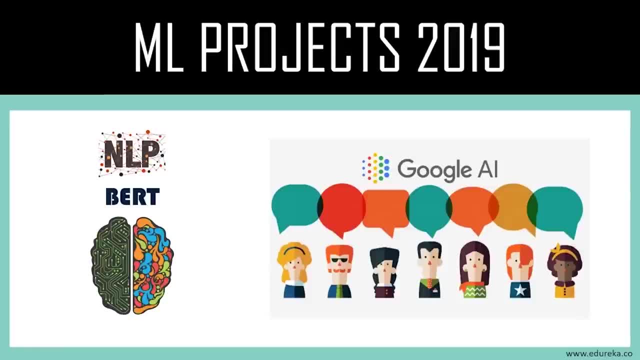 AI's release has smashed record on its way to winning the hearts of NLP enthusiasts and experts alike. following UL, MFIT and ELMO, BRT really blew away the competition with its performance. it obtained the state-of-art result on 11 NLP tasks. apart from the official Google repository, there is a PyTorch. 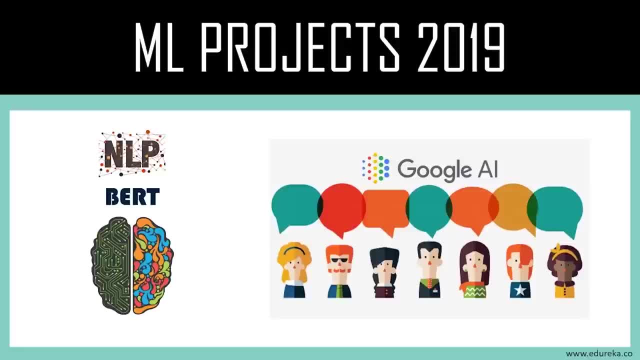 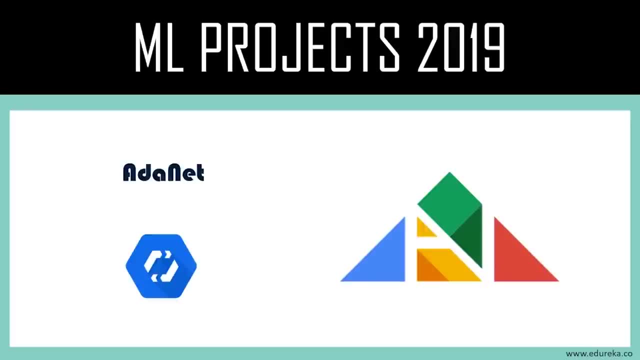 implementation of BERT, which is worth checking out. whether it makes a new era or not in natural language processing we will soon find out. now, Aranet- I'm sure you guys might have heard of it. it is a frame work for automatically learning high quality models without requiring programming expertise, since it's a 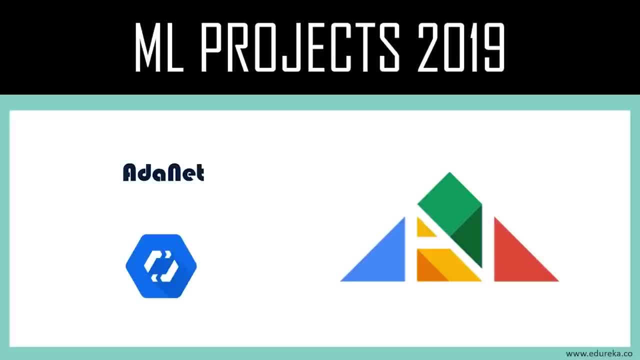 Google invention. the framework is based on tensorflow and you can build ansible models using Aranet and even extend it to use to train a neural network. now the GitHub page contains the code, an example, the API documentation and other things to get your hands dirty. but trust me, auto, auto. 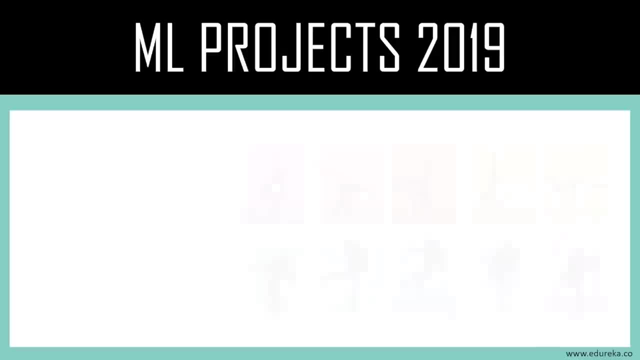 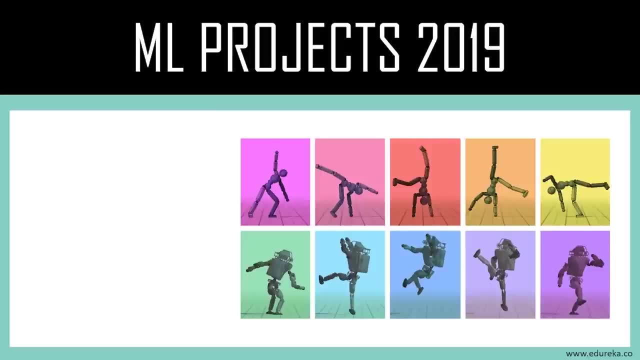 ml is the next big thing in our field. now, if you follow a few researchers on social media, you must have come across some of the images i am showing here in a video form: a stick, human running across the terrain or trying to stand up or some sort. now that my friends is reinforcement learning in. 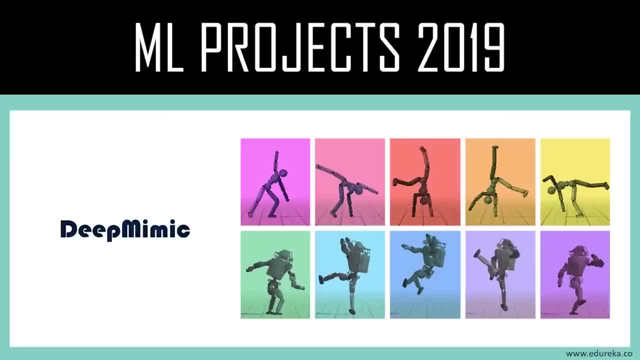 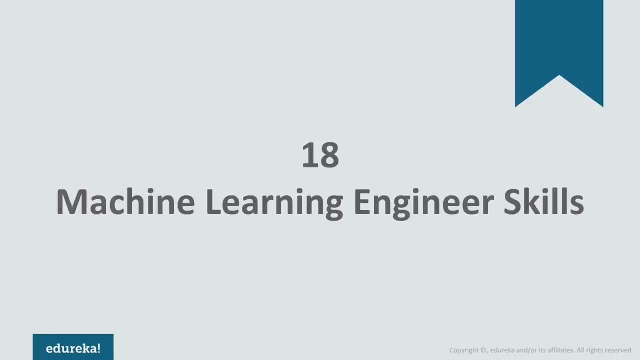 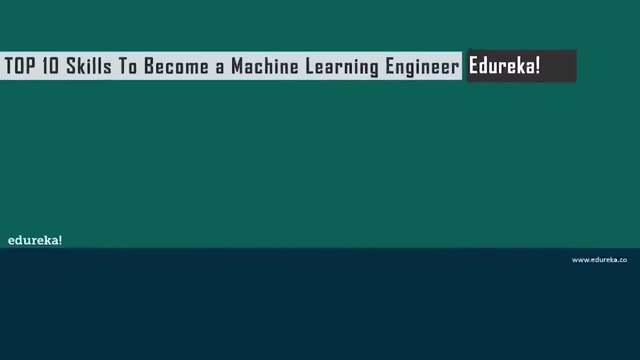 action. now here's a signature example of it: a framework to train a simulated humanoid to imitate multiple motion skill. so let's have a look at the top 10 skills which are required to become a successful machine learning engineer. so, starting with programming languages, python is the lingua. 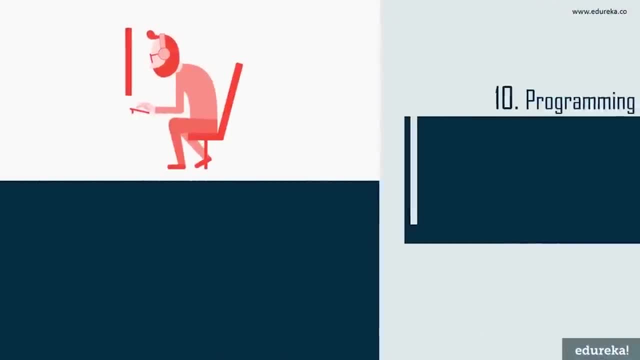 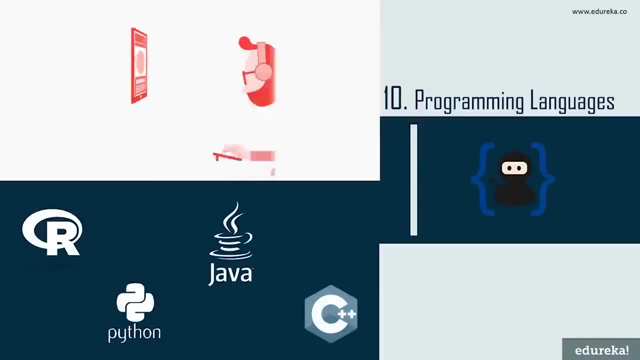 franca of machine learning. you may have had exposure to python, even if you weren't previously in programming or in a computer science related field. however, it is important to have a solid understanding of classes and data structures. sometimes python won't be enough. often you'll encounter projects that need to leverage hardware for speed improvements. now make sure. 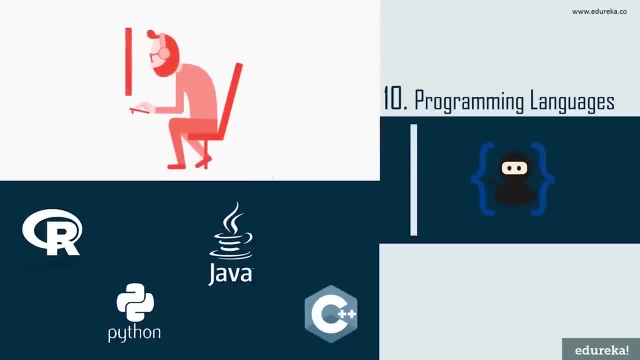 you're familiar with the basic algorithms, as well as the classes, memory, management and linking. now, if you want a job in machine learning, you will probably have to learn all of these languages at some point. c++ can help in speeding code up, whereas r works great in statistics and plots. 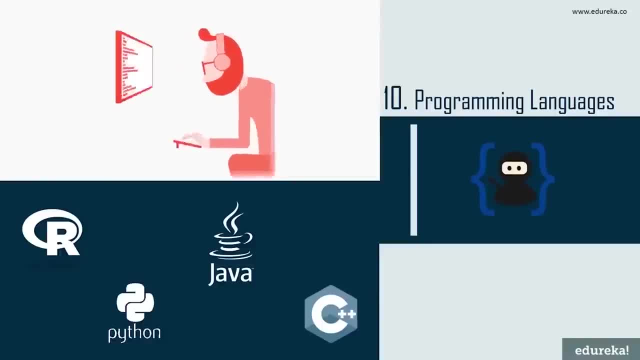 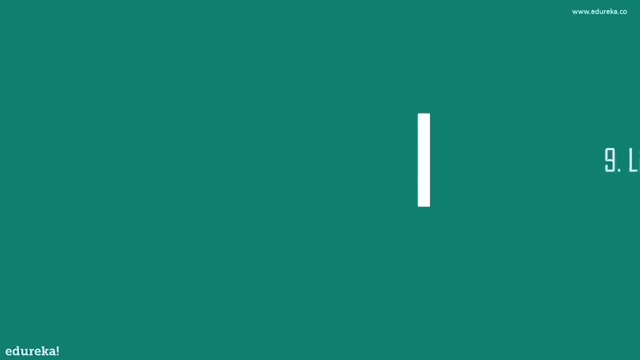 machine learning. you will probably have to learn all of these languages at some point. c++ can help in speeding code up, whereas r works great in statistics and plots, and hadoop is java based, so you probably need to implement mappers and reducers in java now. next we have linear algebra. 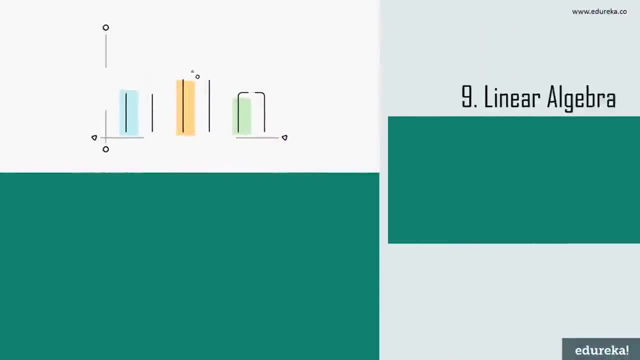 you'll need to be intimately familiar with matrices vectors and matrix multiplication. if you have a lot of knowledge about matrices, you'll need to be familiar with matrices vectors and matrices integrals, and you will have an understanding of derivatives and integrals. you should be in the clear, otherwise even simple concept like gradient descents will elude you. 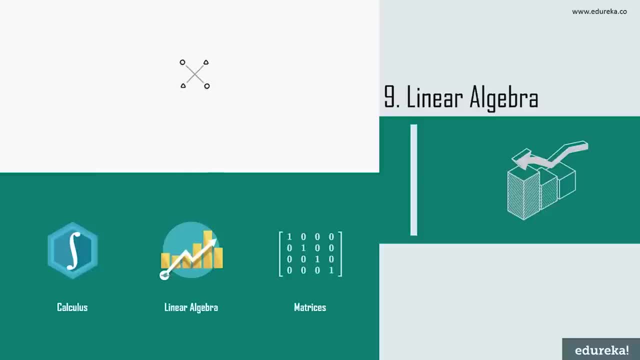 statistic is going to come up a lot. at least make sure you are familiar with the caution. distributions means standard deviation and much more. every bit of statistical understanding beyond this helps. the theory is help in learning about algorithms. grade samples are naive, bias, Gaussian mixture models, a firm understanding of probability and stats to understand these models, Just go nuts and study. 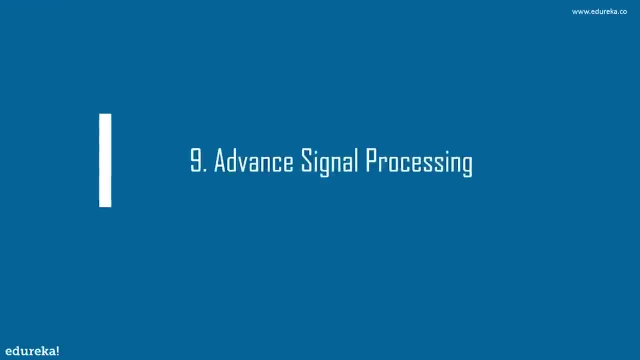 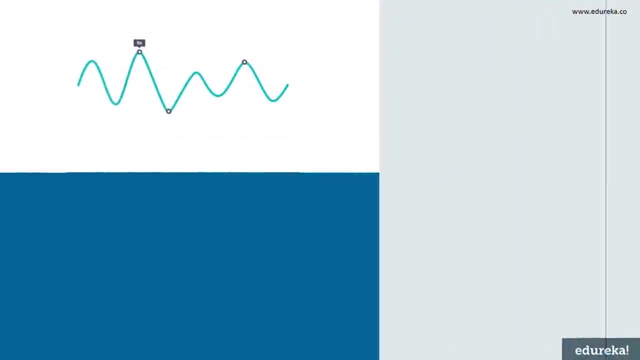 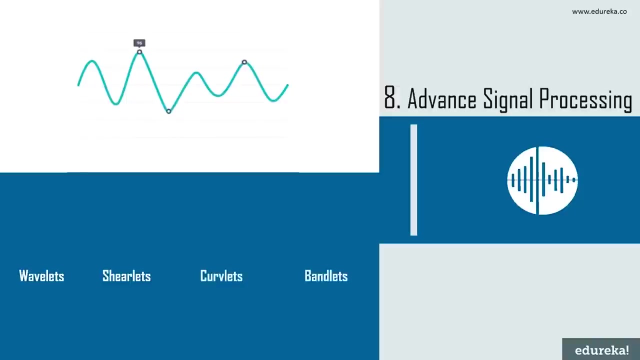 measure theory And next we have advanced signal processing techniques. Now, feature extraction is one of the most important parts of machine learning. Different types of problems need various solutions. You may be able to utilize really cool advanced signal processing algorithms such as wavelets, shearlets, curvelets and bandlets. You need to learn about the time. 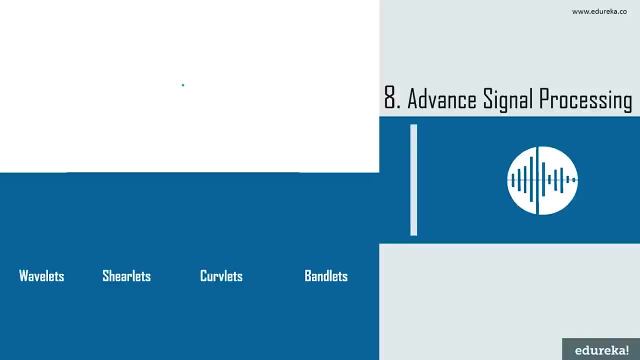 frequency analysis and try to apply it in your problems. Now this skill will give you an edge over all the other skills. Now this skill will give you an edge, while you're applying for a machine learning engineer job, over others. Now next, we have applied maths, A lot of machine. 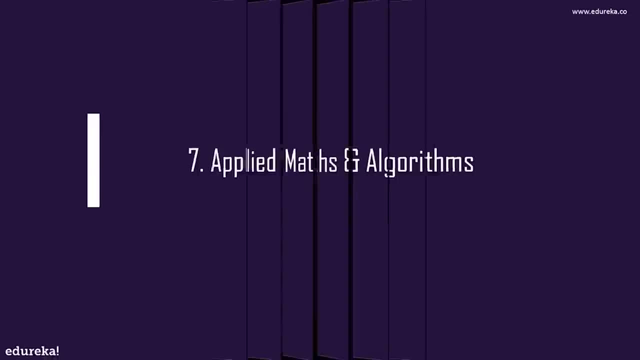 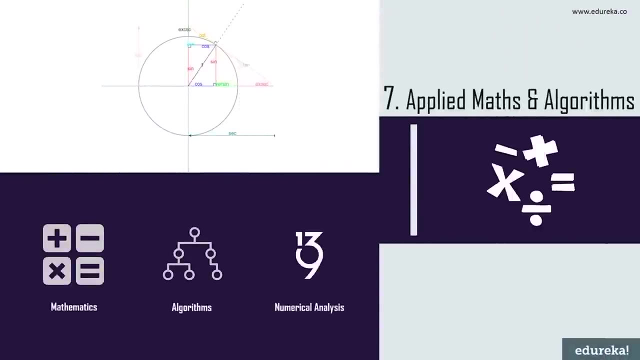 learning techniques out. there are just fancy types of functional approximation. Now these often get developed by theoretical mathematician and then get applied by people who do not understand the theory at all. Now the result is that many developers might have a hard time finding the best way to solve the problem. Now this skill will give you an edge over all the. 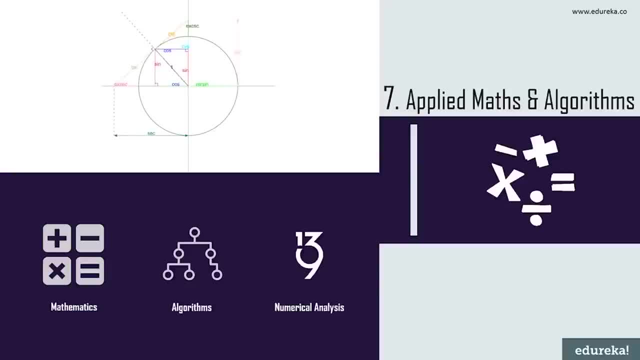 best techniques for the problem. So even a basic understanding of numerical analysis will give you a huge edge. Having a firm understanding of algorithm theory and knowing how the algorithm works, you can also discriminate models such as SVMs. Now you will need to understand subjects. 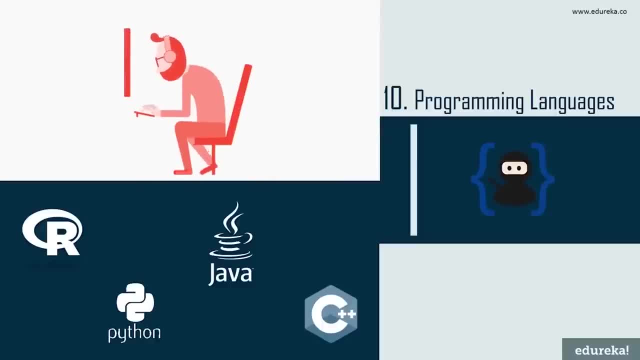 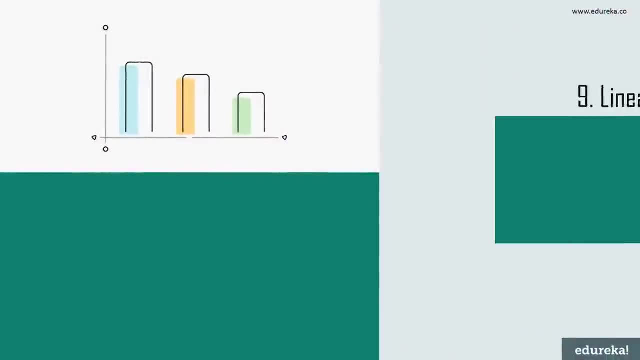 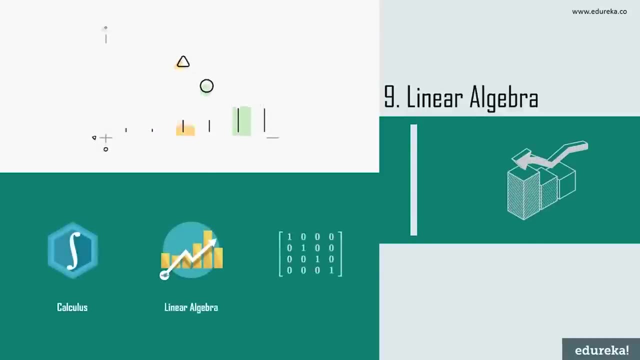 and hadoop is java based, so you probably need to implement mappers and reducers in java now. next we have linear algebra. you'll need to be intimately familiar with matrices, vectors and matrix multiplication. if you have an understanding of derivatives and integrals, you should be in the clear. otherwise, 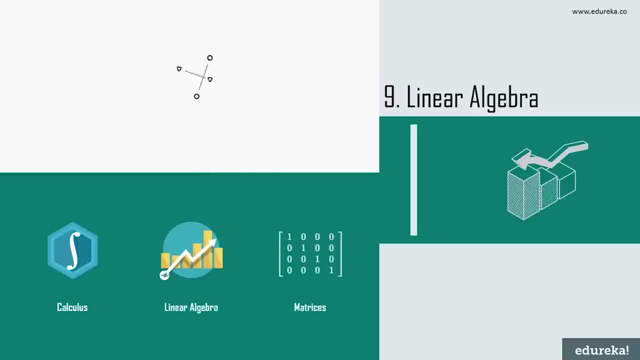 even simple concept like gradient descents will elude you. statistic is going to come up a lot. at least make sure you are familiar with the caution. distributions means standard deviation and much more. every bit of statistical understanding beyond this helps. the theories help in learning about algorithms. great samples are. 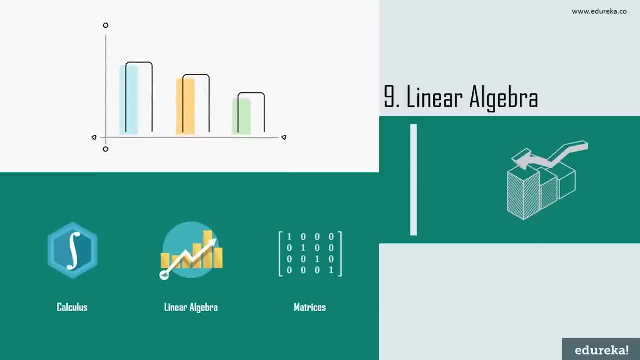 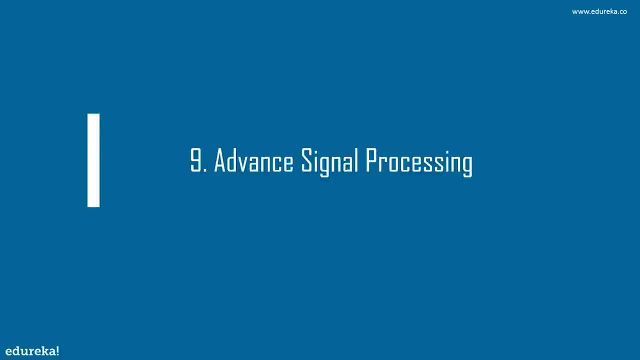 naive bias, caution mixture models and hidden markup models. you need to have a firm understanding of probability and stats to understand these models. just go nuts and study measure theory and next we have advanced signal processing techniques now feature abstraction is one of the most important parts of machine learning. different types of problems need various solutions. you may be able. 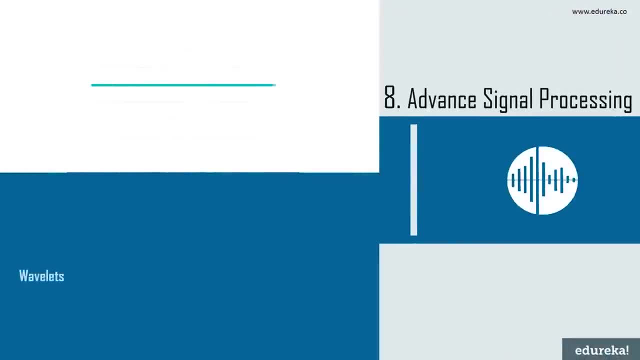 to utilize really cool advanced signal processing algorithms such as wavelets, she alerts, coblet and and bandless. you need to learn about the time frequency analysis and try to apply it in your problems now. this skill will give you an edge over all the other skills. now, this skill will give you an edge. 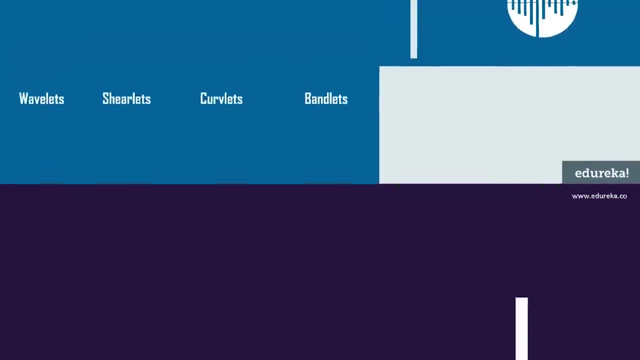 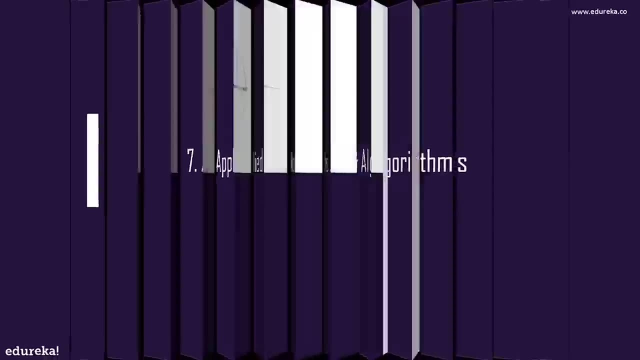 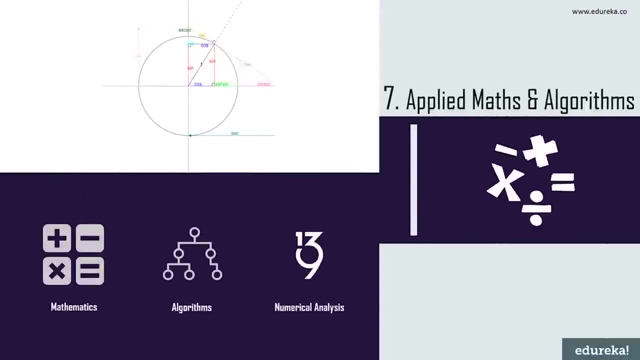 while you are applying for a machine learning engineer job over others. now next, we have applied maths, a lot of machine learning techniques out. there are just fancy types of functional approximation. now. these often get developed by theoretical mathematician and then get applied by people who do not understand the theory at all. 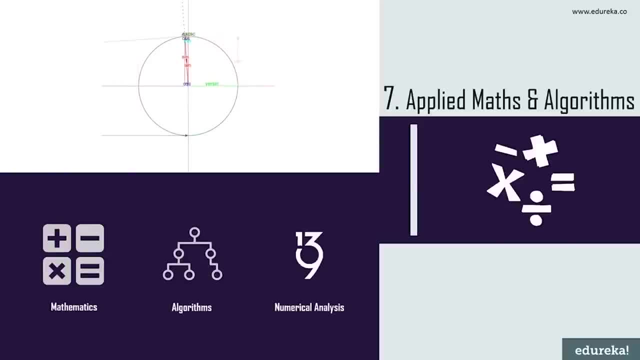 now. the result is that many developers might have a hard time finding the best techniques for the problem. so even a basic understanding of numerical analysis will give you a huge edge. having a firm understanding of algorithm theory and knowing how the algorithm works, you can also discriminate models such as: 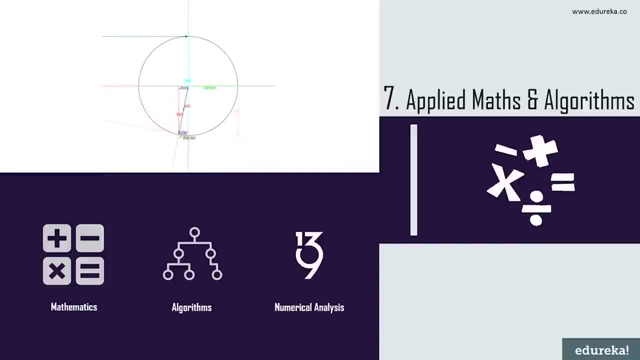 svms. now you will need to understand subjects such as gradient, descent, convex optimization, lag range, quadratic programming, partial differentiation equations and much more. now, all this math might seem intimidating at first if you have been away from it for a while. yes, machine learning is much more math intensive than something like front-end. 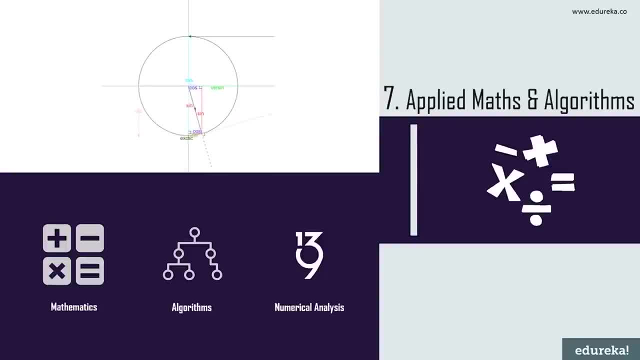 such as gradient descent, convex optimization, lag range, quadratic programming, partial differentiation equations and much more. Now, all this math might seem intimidating at first if you have been away from it for a while. Yes, machine learning is much more math intensive than something like front-end development. 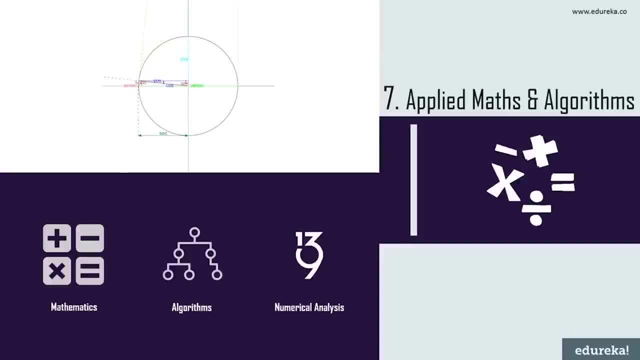 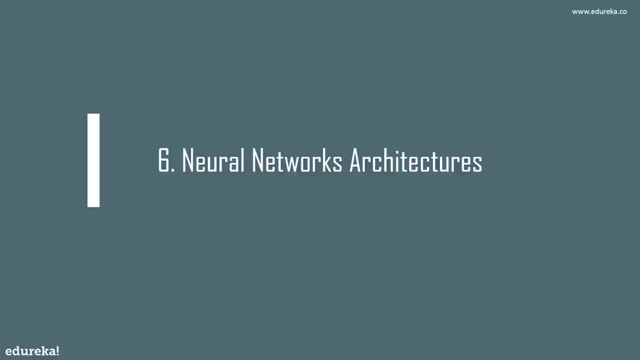 Just like any other skill, getting better at math is a matter of focused practice. Now, next skill in our list is the neural network architectures. We need machine learning for tasks that are too complex for human to code directly, That is, tasks that are so complex. 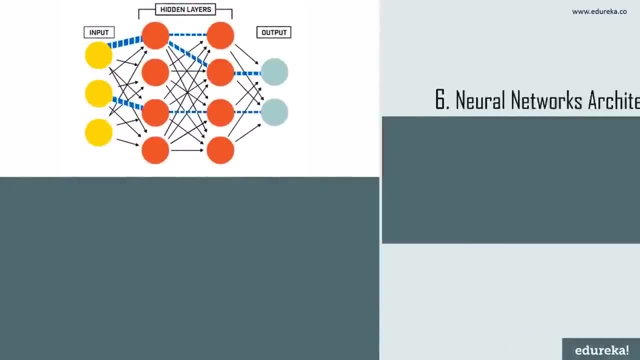 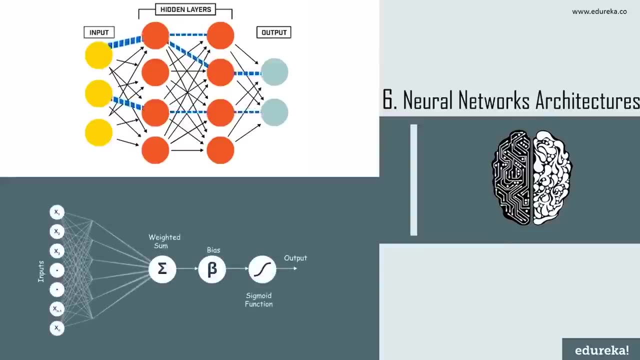 that it is impractical. Now neural networks are a class of models within the general machine learning literature. Now neural networks are a specific set of algorithms that have revolutionary, revolutionized machine learning. They are inspired by biological neural networks and the current so-called deep neural networks have proven to work quite well. The neural 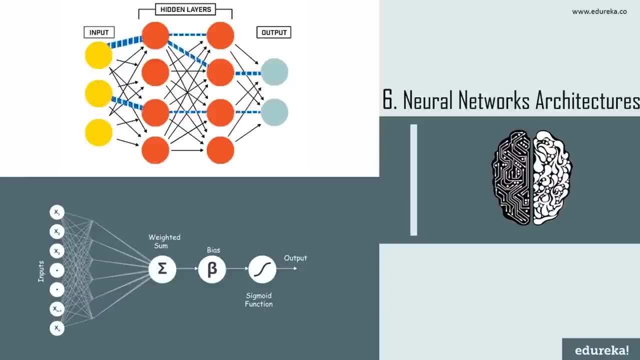 networks are themselves general function approximations, which is why they can be applied to almost any machine learning problem about learning a complex mapping from the input to the output space. Of course there are still good reasons for the surge in the popularity of neural networks, But neural networks have been by far the most accurate way of approaching many 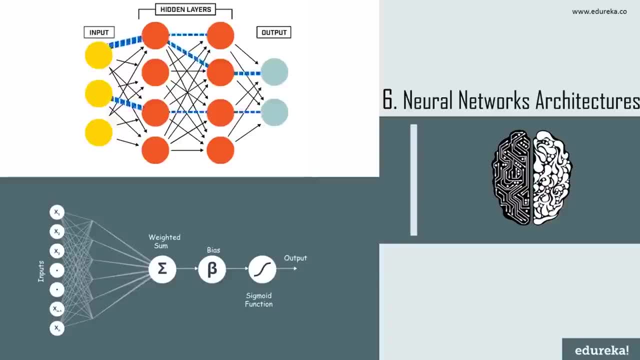 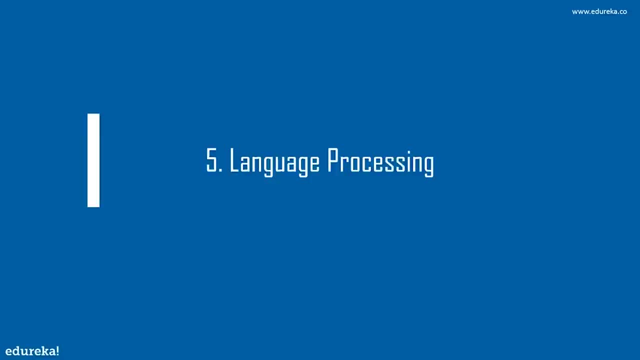 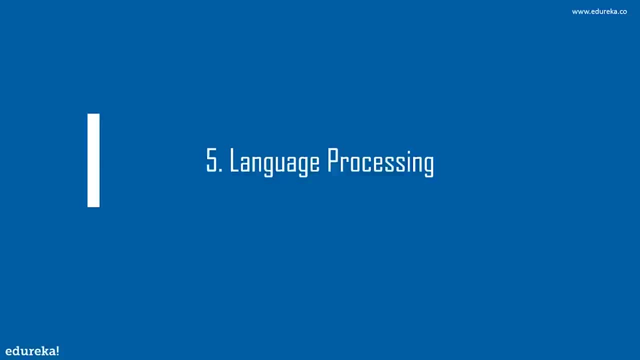 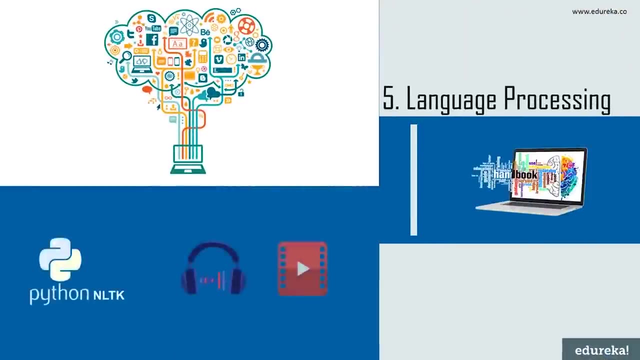 Genesysm and the techniques, such as sentimental analysis and summarization, that are unique to NLP. Now, audio and video processing has a frequent overlap with the natural language processing. However, natural language processing can be applied to non-audio data like text. 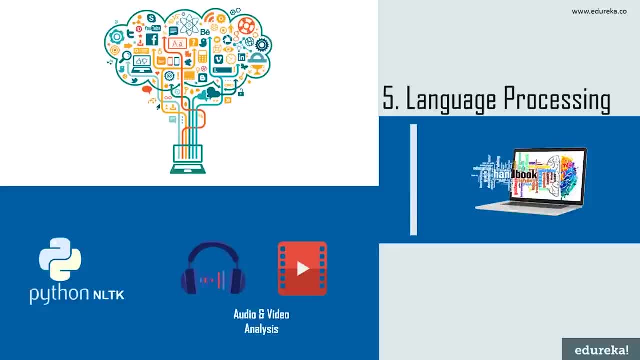 sentences and words, extracting useful information from the audio signals themselves. Being well-versed in math will get you far in this one, And you should also be familiar with the concepts such as the fast Fourier transforms. Now, these were the technical skills that are required to become a successful machine learning. 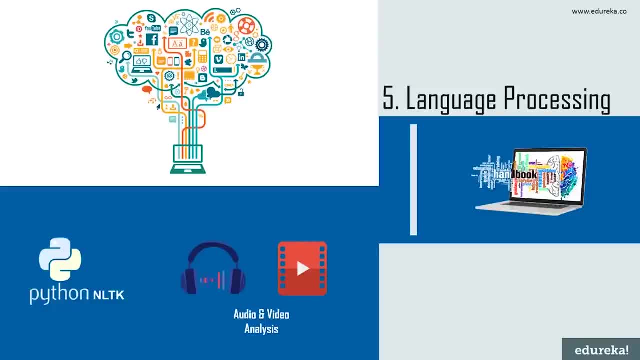 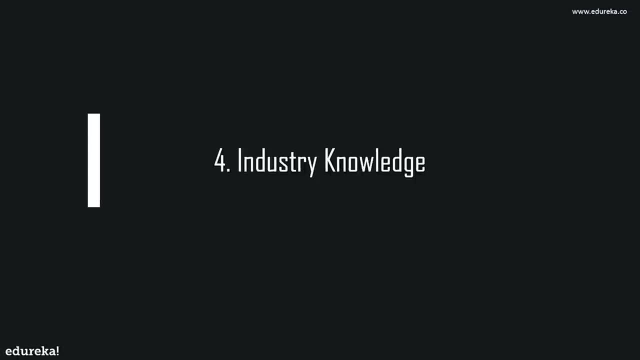 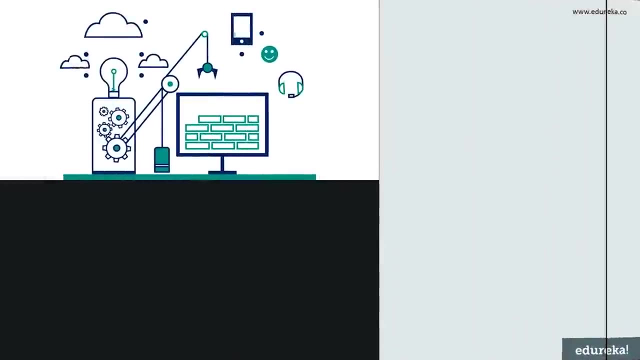 engineer. So next I'm going to discuss some of the non-technical skills, or the soft skills which are required to become a machine learning engineer. So first of all we have the industrial knowledge. Now, the most successful machine learning projects out there are going to be those that address real pain points. whichever industry you 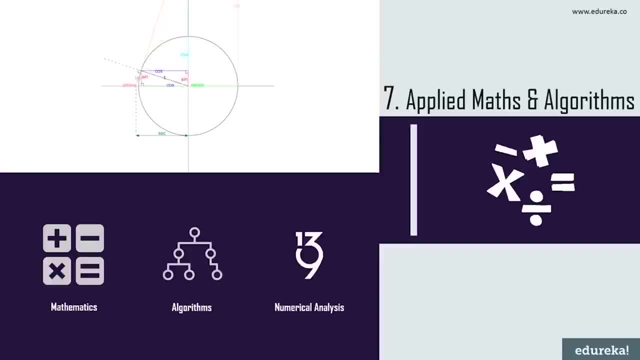 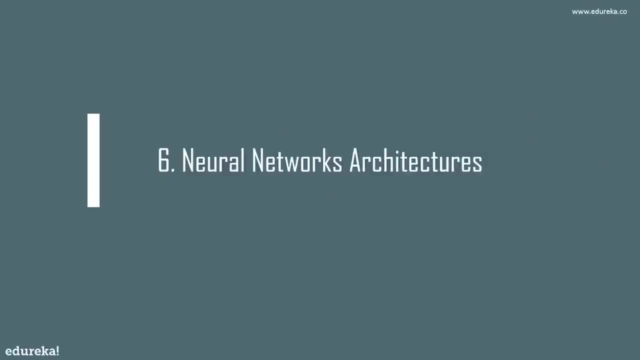 development, just like any other skill. getting better at math is a matter of focus, practice. the next skill in our list is the neural network architectures. we need machine learning for tasks that are too complex for human to code directly, that is, tasks that are so complex that it is impractical. 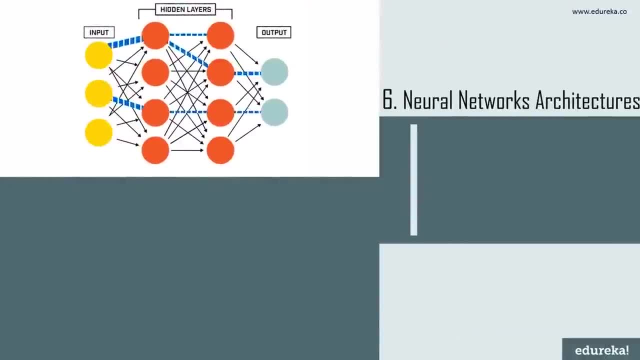 now, neural networks are a class of models within the general machine learning literature. neural networks are a specific set of algorithms that have revolutionized machine learning. they are inspired by biological neural networks, and the current so-called deep neural networks have proven to work quite well. the neural networks are themselves general function approximations, which is 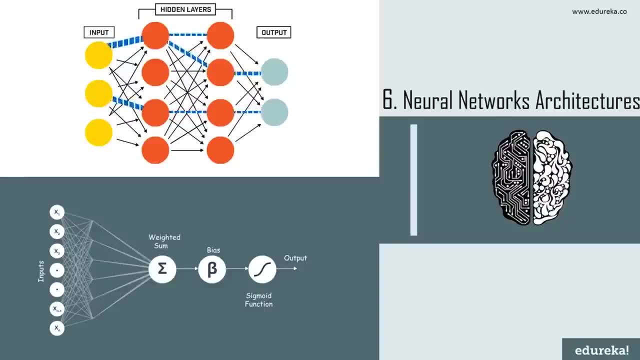 why they can be applied to almost any machine learning problem about learning a complex mapping from the input to the output space. of course, there are still good reasons for the surge in the popularity of neural networks, but neural networks have been by far the most accurate way of approaching many problems like 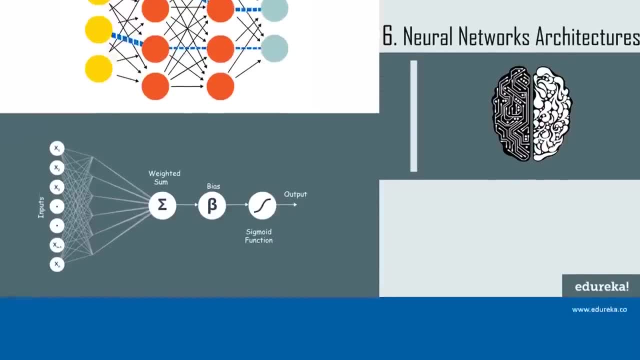 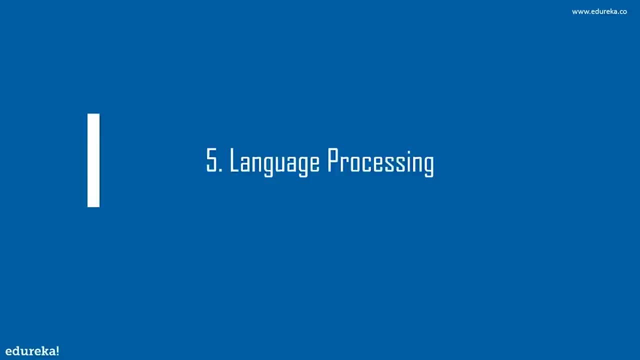 translation, speech recognition and image classification. now coming to our next point, which is the natural language processing now, since it combines computer science and linguistic. there are a bunch of libraries like the nltk, genesism and the techniques, such as sentimental analysis and summarization, that are unique to nlp. now, 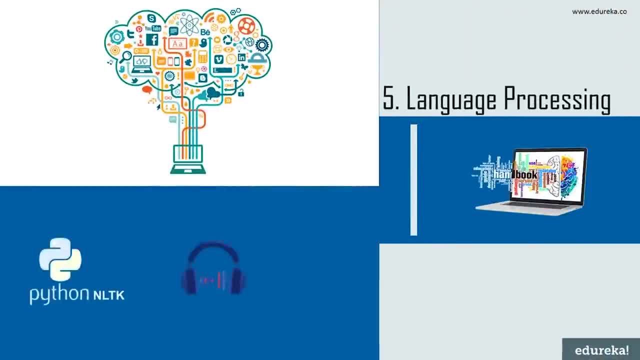 audio and video processing has a frequent overlap with the natural language processing. however, natural language processing can be applied to non-audio data like text, voice, and audio analysis involves extracting useful information from the audio signals themselves. Being well versed in math will get you far in this one, and you should. 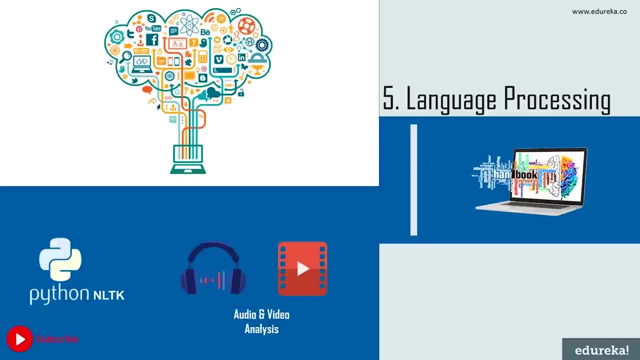 also be familiar with the concepts such as the fast Fourier transforms. Now, these were the technical skills that are required to become a successful machine learning engineer. So next I'm going to discuss some of the non-technical skills, or the soft skills, which are required to become 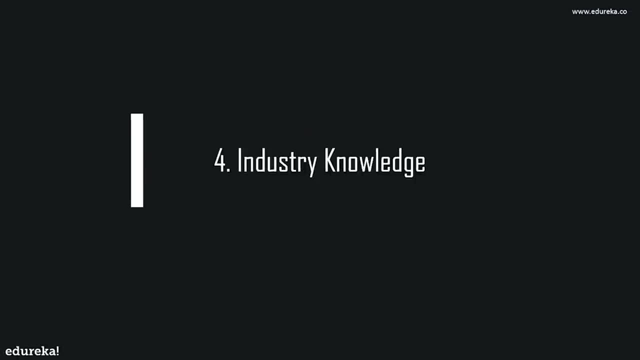 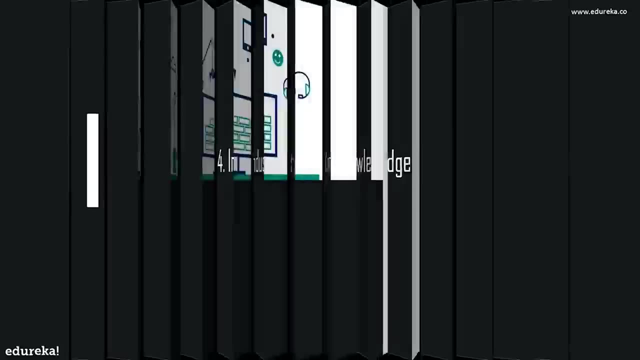 a machine learning engineer. So first of all, we have the industry knowledge. Now, the most successful machine learning projects out there are going to be those that address real pain points. Whichever industry you are working for, you should know how that industry works and what will be beneficial. 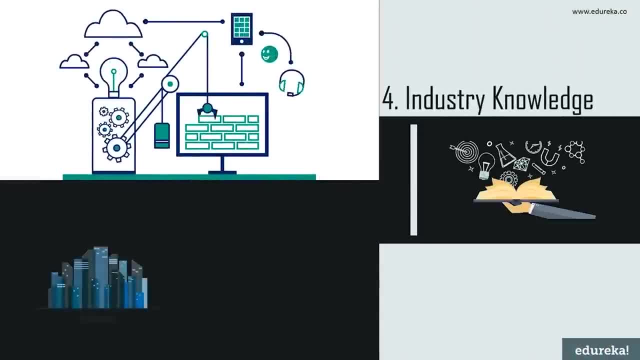 are working for you should know how that industry works and what will be beneficial for the business. if a machine learning engineer does not have business acumen and the know-how of the elements that make up a successful business model or any particular algorithm, then all those technical 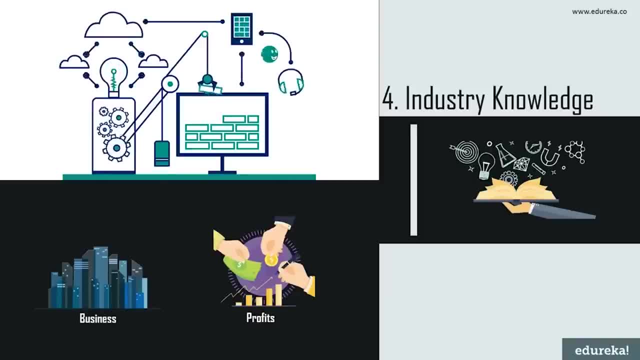 skills cannot be channeled productively. you won't be able to discern the problems and potential challenges that need solving for the business to sustain and grow. you won't really be able to help your organization explore new business opportunities. so this is a must-have skill now. next, we have 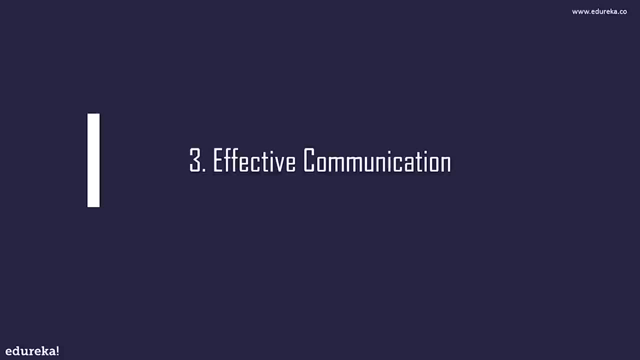 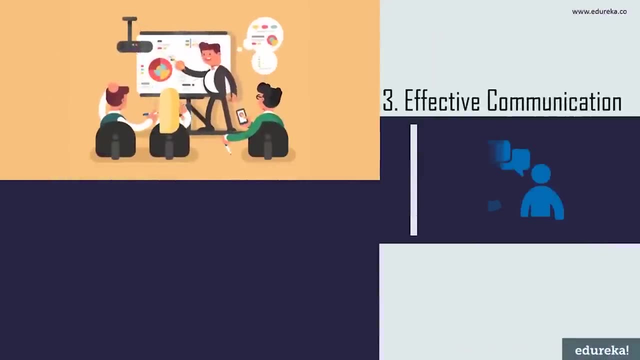 effective communication. now you'll need to explain the machine learning concepts to the people with little to no expertise in the field. chances are you'll need to work with a team of engineers, as well as many other teams, so communication is going to make all of this much more easier. 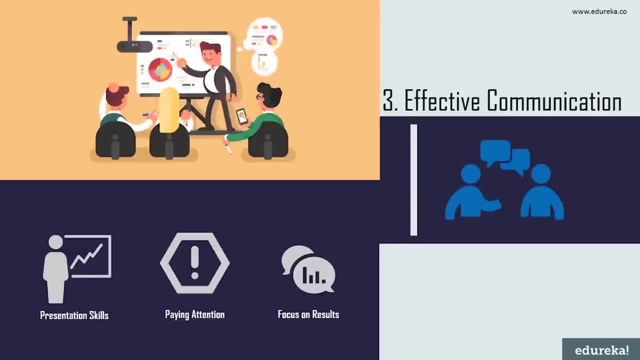 companies searching for a strong machine learning engineer are going to need to be able to explain the concepts to the people with little to no expertise in the field, looking for someone who can clearly and fluently translate their technical findings to a non-technical team such as marketing or sales department. now, next on our list, we have rapid. 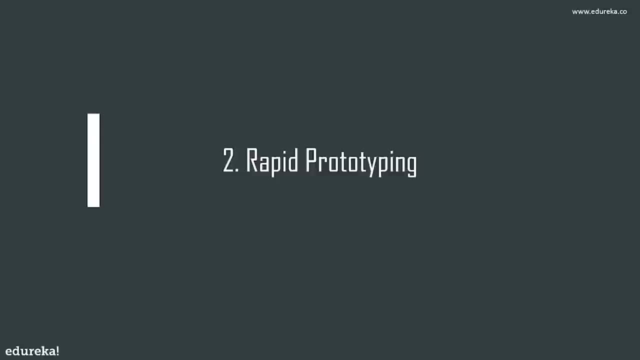 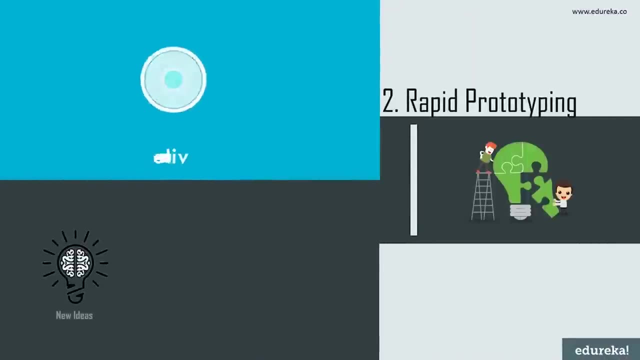 prototyping, so iterating on ideas as quickly as possible is mandatory for finding one that works in machine learning. this applies to everything from picking up the right model to working on projects such as a- b testing. you need to do a group of techniques used to quickly fabricate a scale. 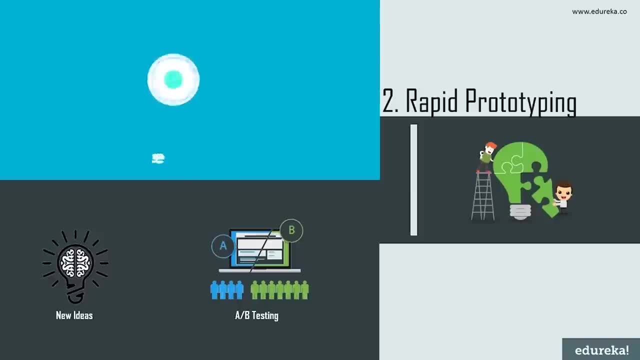 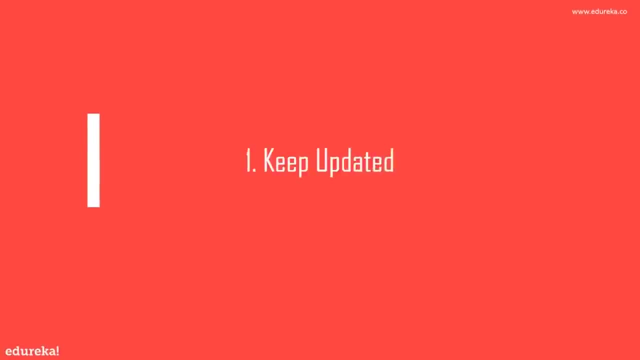 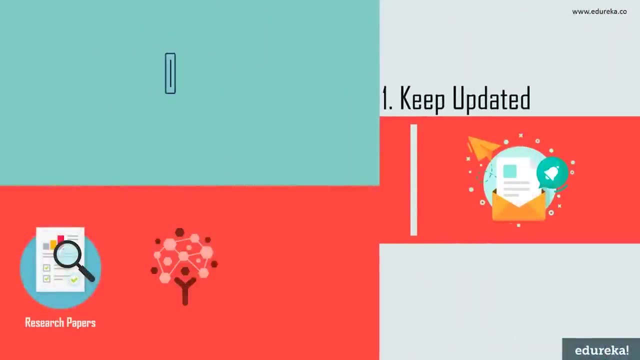 model of a physical part or assembly using the three-dimensional computer-aided design which is the cad. so, last but not the least, we have the final skill, and that is to keep updated. you must stay up to date with any upcoming changes. every month, new neural network models come out that 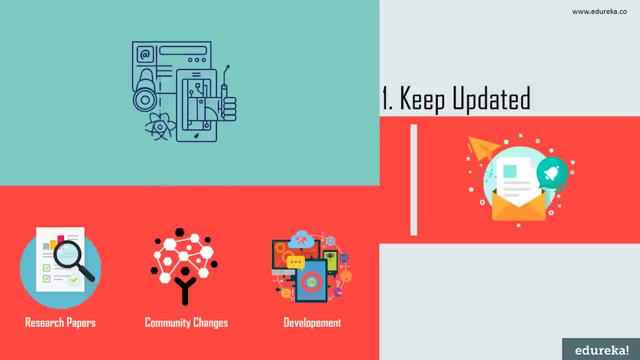 outperform the previous architecture. it also means being aware of the news regarding the development of the tools, the change log, the conferences and much more. you need to know about the theories and algorithms now. let's get started now. this you can achieve by reading the research papers, blogs, the conferences, videos and also you. 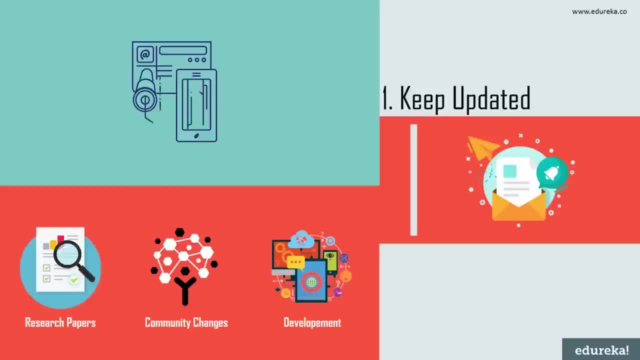 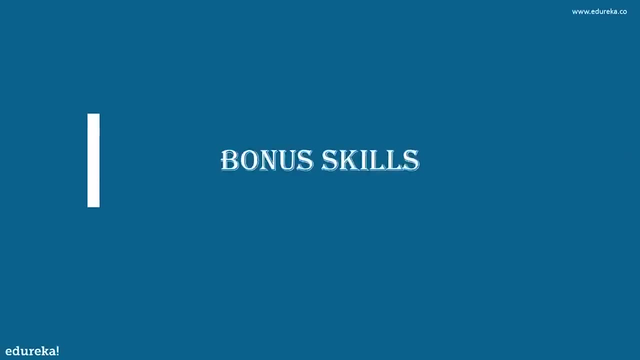 need to focus on the online community with changes very quickly, so expect and cultivate this change now. this is not the end here. we have certain skills, the bonus skills, which will give you an edge over other competitors or the other persons who are applying for a machine learning. 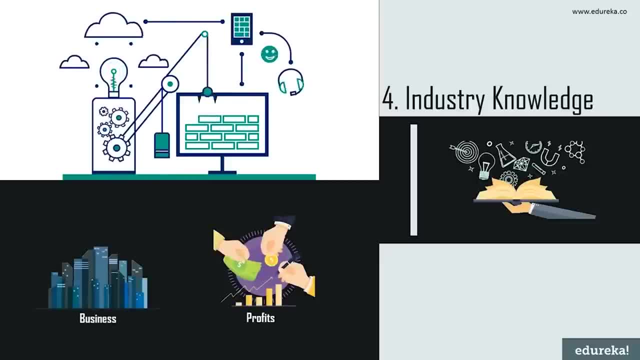 for the business. If a machine learning engineer does not have business acumen and the know-how of the elements that make up a successful business model or any particular algorithm, then all those technical skills cannot be channeled productively. You won't be able to discern the problems and potential challenges that need solving for the 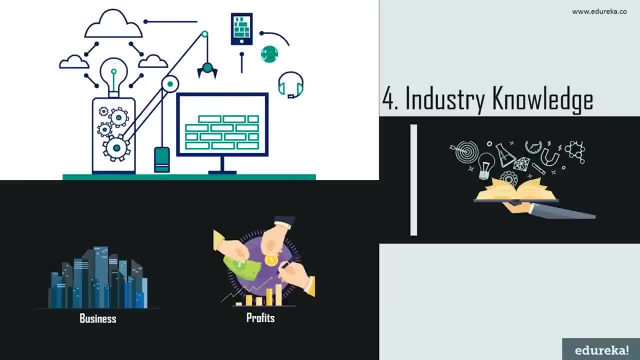 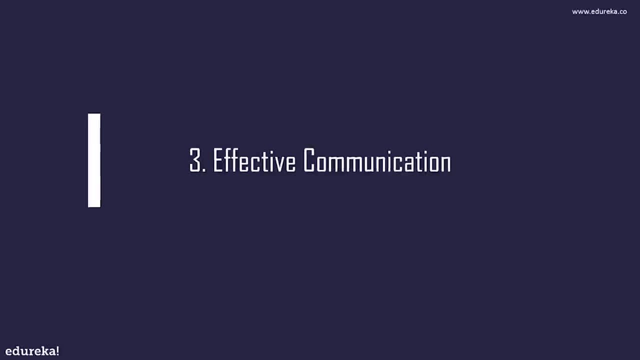 business to sustain and grow, You won't really be able to help your organization explore new business opportunities, So this is a must-have skill Now. next, we have effective communication. You'll need to explain the machine learning concepts to the people with little to no expertise in the field. 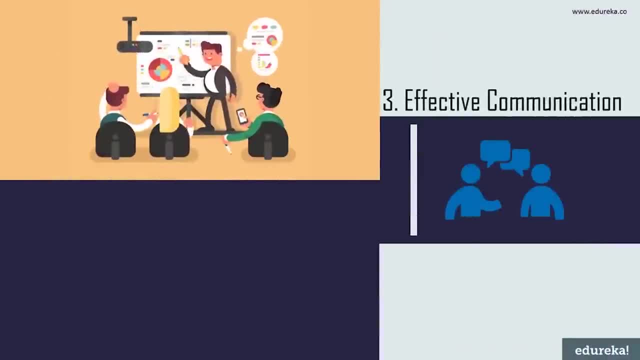 Chances are, you'll need to work with a team of engineers, as well as many other teams, So communication is going to make all of this much more easier. Companies searching for a strong machine learning engineer are looking for someone who can clearly and fluently translate their technical findings to a non-technical team, such as marketing or sales. 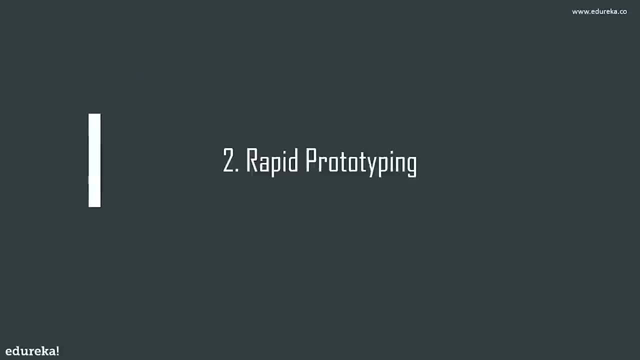 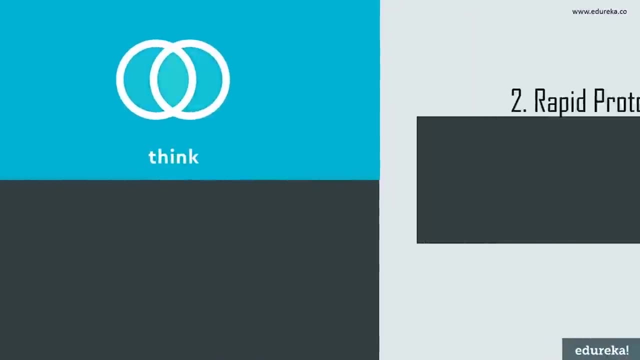 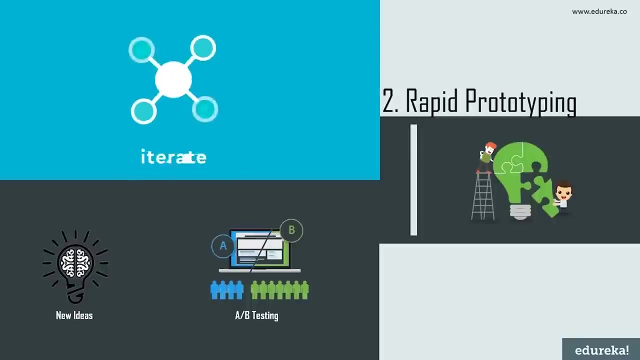 department. Now next on our list, we have rapid prototyping, So iterating on ideas as quickly as possible is mandatory for finding one that works In machine learning. this applies to everything from picking up the right model to working on projects such as A-B testing. You need to do a group of 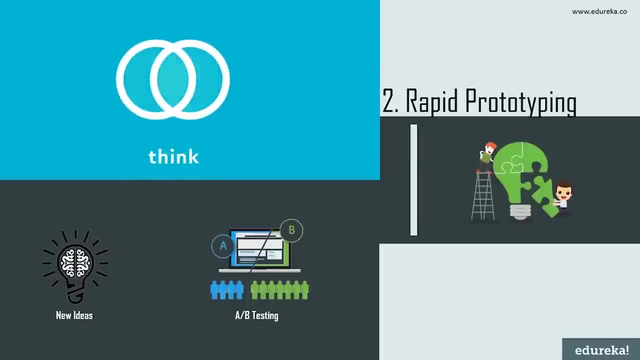 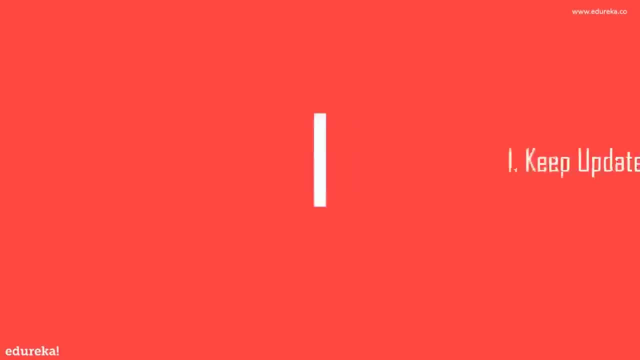 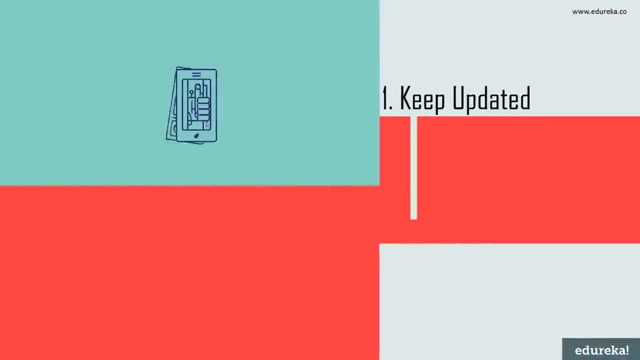 techniques used to quickly fabricate a scale model of a physical part or assembly using the three-dimensional computer-aided design which is the CAD. So, last but not the least, we have the final skill, and that is to keep updated. You must stay up to date with any upcoming changes Every. 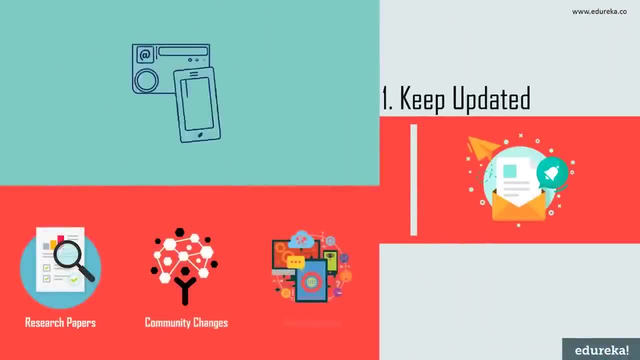 month, new neural network models come out that outperform the previous architecture. It also means being aware of the news regarding the development of the tools, the change log, the conferences and much more. You need to know about the theories and algorithms Now. this you can achieve by reading the research. 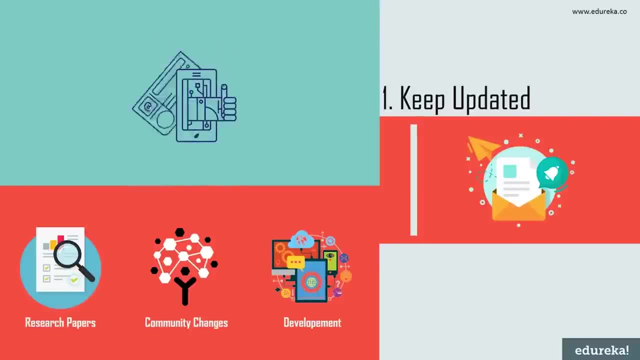 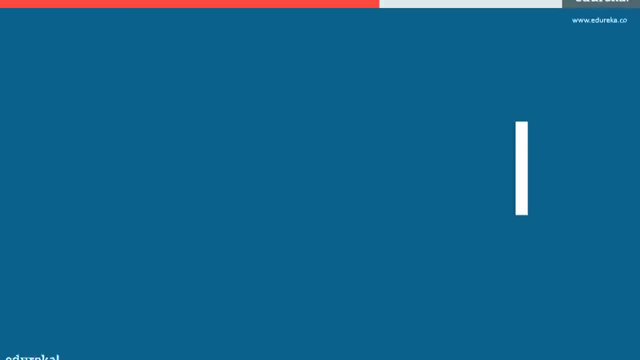 papers, blogs, the conferences, videos, and also you need to focus on the online community with changes very quickly, So expect and cultivate this change Now. this is not the end Here. we have certain skills, The bonus skills, which will give you an edge over other competitors or the other persons. 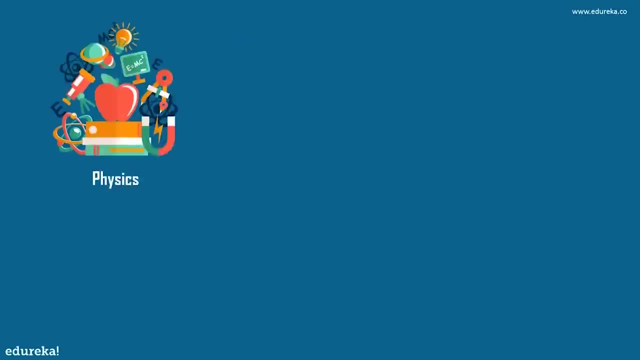 who are applying for a machine learning engineer position. On the bonus point, we have physics. Now you might be in a situation where you would like to apply machine learning techniques to a system that will interact with the real world. Having some knowledge of physics will take you far Now. next we have reinforcement learning. So this reinforcement- 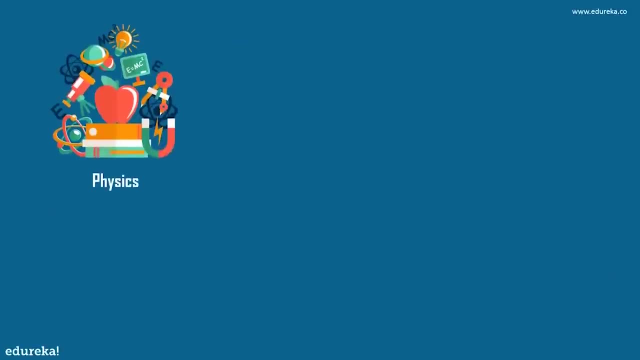 engineer position. on the bonus point, we have physics. now you might be in a situation where you would like to apply machine learning techniques to a system that will interact with the real world. having some knowledge of physics will take you far now. next we have reinforcement learning, so this reinforcement learning has been a driver behind many of the most 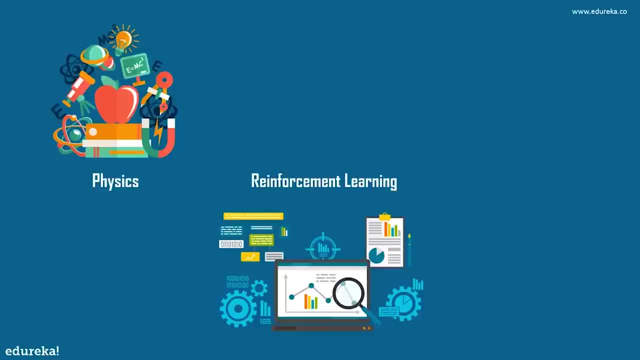 exciting developments in the deep learning and the ai community, from the alpha go zero to the open ai's dota 2, but this will be a critical to understand if you want to go into robotics, self-driving cars or other ai related areas. and finally we have computer vision. out of all the 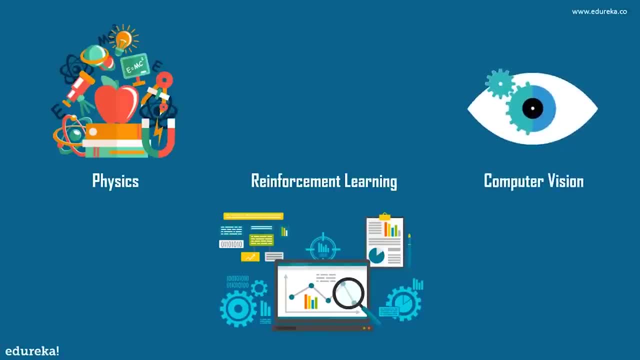 disciplines out there. there are by far the most resources available to you in terms of computer vision. there are by far the most resources available to you in terms of computer vision. there are by far the most resources available for learning computer vision. this field appears to have the lowest. 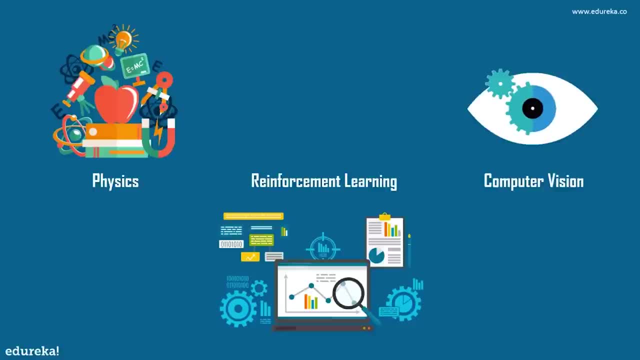 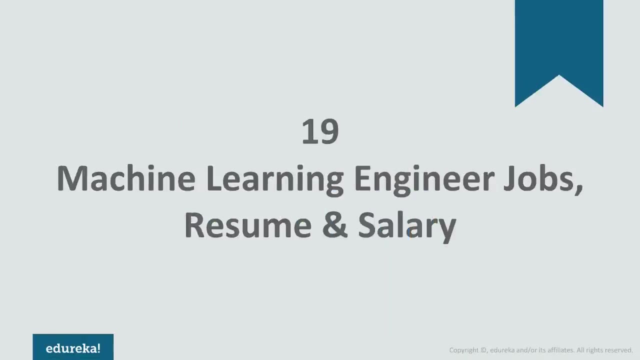 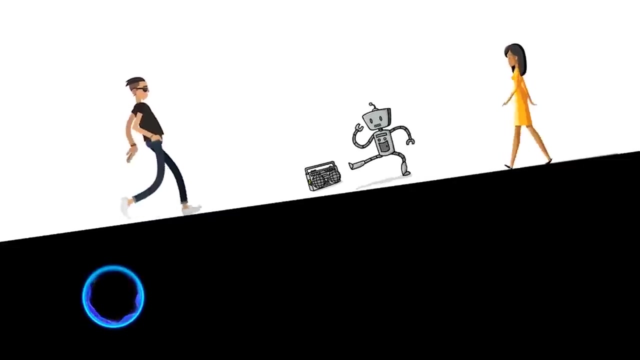 barriers to entry, but of course this likely means you'll face slightly more competition. so having a good knowledge of computer vision, how it works, will give you an edge over other competitors. now i hope you got acquainted with all the skills which are required to become a successful machine learning engineer. as you know, we are living in the worlds of humans and machines. 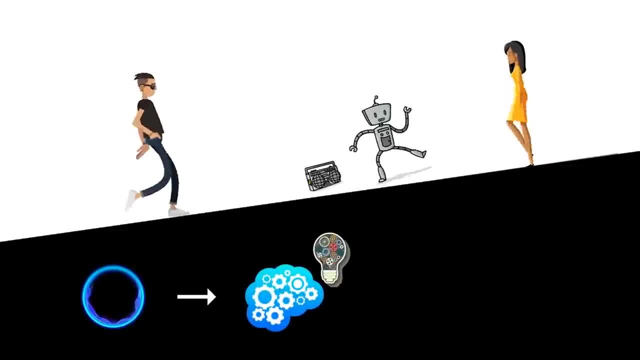 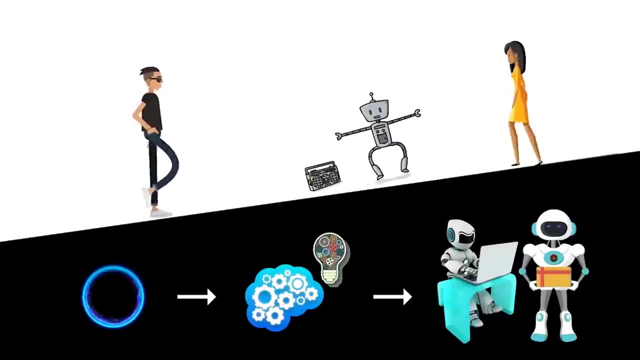 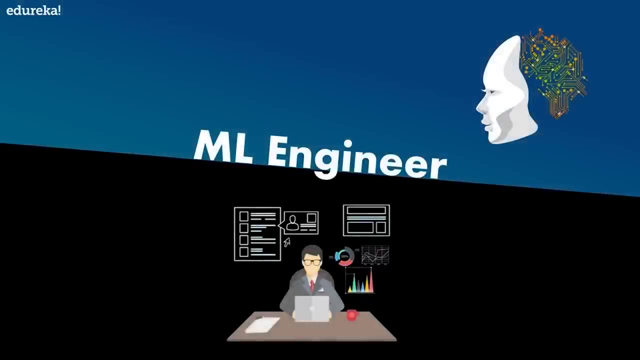 these machines or the robots have to be programmed before they start following your instructions. but what if the machines started learning on its own from their experience, work like us and feel like us and do things more accurately than us now? well, here's where a machine learning engineer comes into picture to make sure everything is working according to. 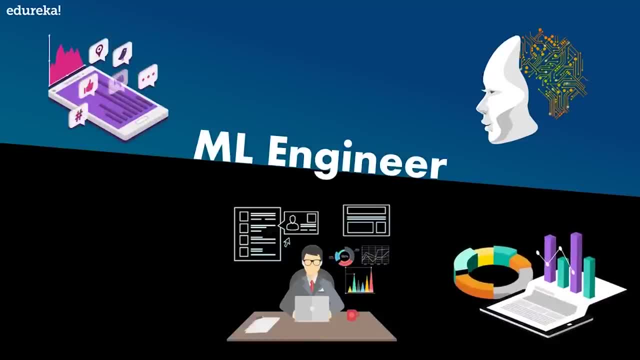 the procedures and the guidelines. now, in my opinion, machine learning is one of the most recent and exciting technologies there is. you probably use it a dozen of times every day without knowing it. so before we indulge into the different roles, the salary trends and what should be there, 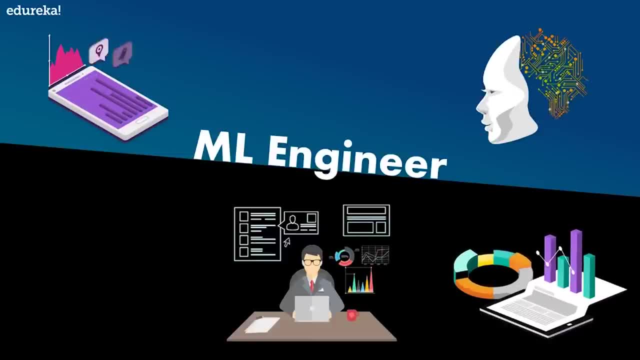 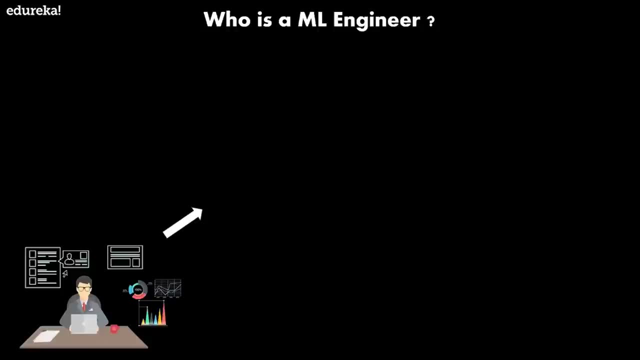 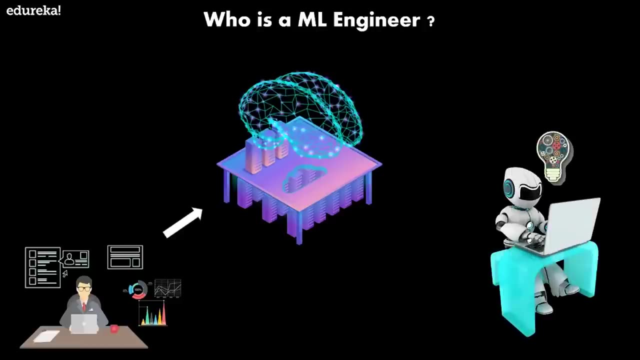 on the resume of a machine learning engineer while applying for a job. let's understand who exactly a machine learning engineer is. so machine learning engineers are sophisticated programmers who develop machines and systems that can learn and apply knowledge without specific direction. artificial intelligence is the goal of a machine learning engineer. they are computer programmers. 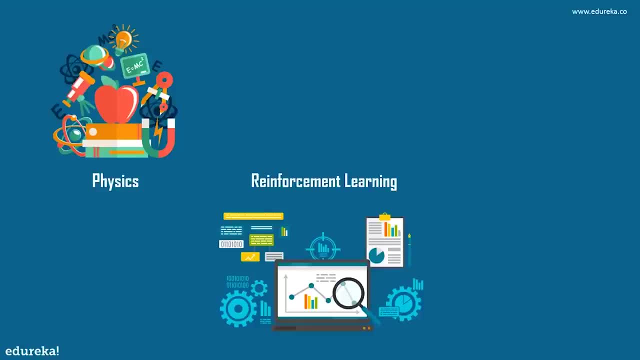 learning has been a driver behind many of the most exciting developments in the deep learning and the AI community, From the alpha go zero to the open AI's dota 2. but this will be a critical to understand if you want to go into robotics, self-driving cars or other AI related areas. And finally, we have 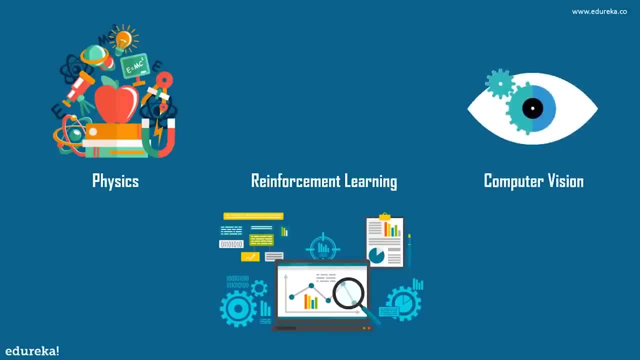 computer vision. Out of all the disciplines out there, there are by far the most resources available for learning computer vision. This field appears to have the lowest barriers to entry, but of course this likely means you'll face slightly more competition. So having a good knowledge of computer vision, how it works, will give you an edge. 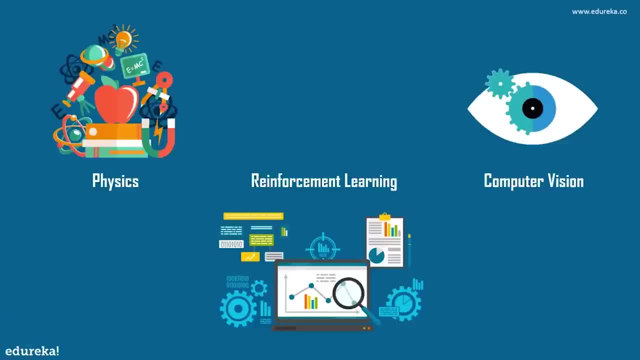 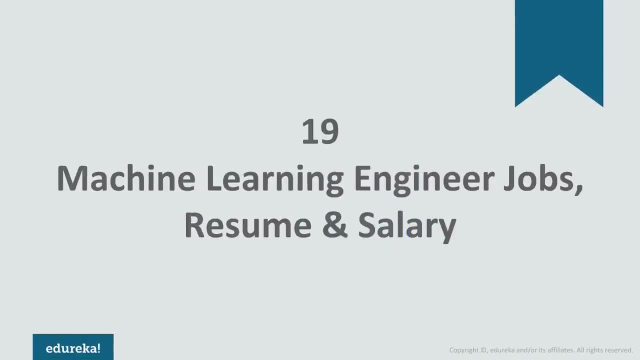 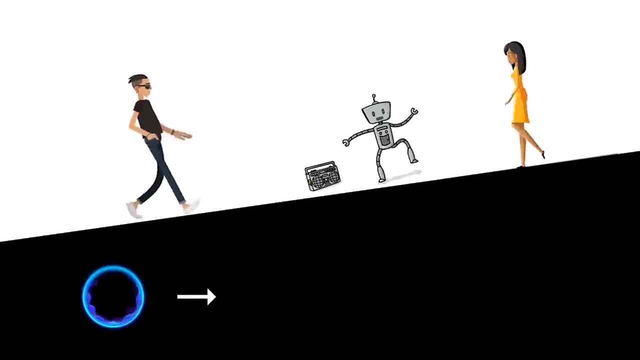 over other competitors. Now I hope you got acquainted with all the skills which are required to become a successful machine learning engineer. As you know, we are living in the world of humans and machines. In today's world, these machines, or the robots, have to be programmed. 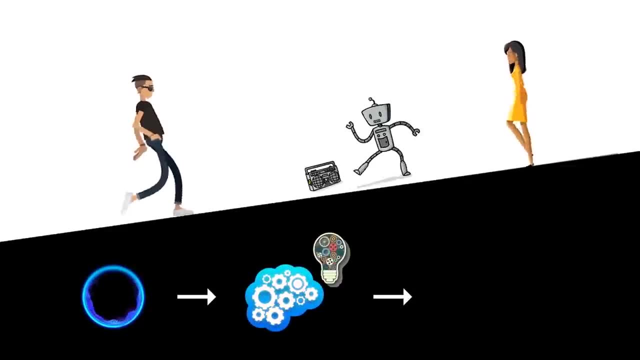 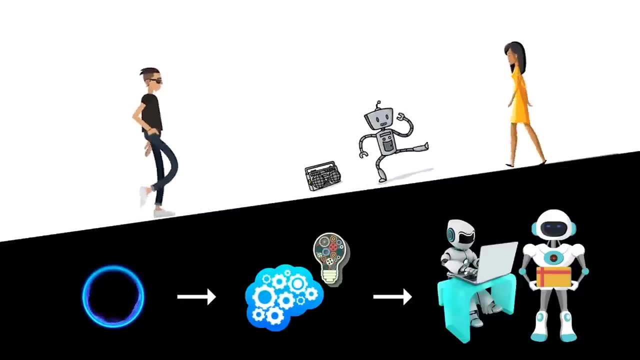 before they start following your instructions. But what if the machines started learning on its own from their experience, work like us and feel like us and do things more accurately than us? Now, well, here's where a machine learning engineer comes into picture to make sure everything. 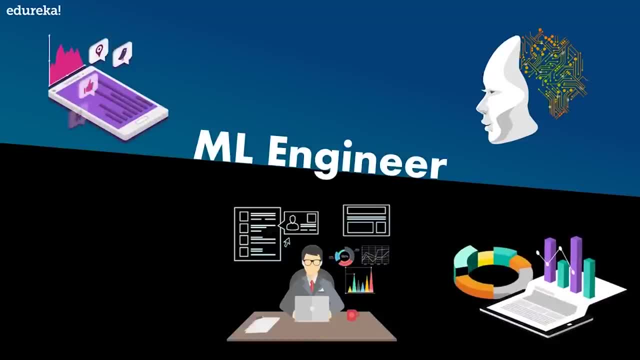 is working according to the procedures and the guidelines. Now, in my opinion, machine learning is one of the most recent and exciting technologies there is. We use it a dozen of times every day, without even knowing it. So, before we indulge into the different roles, the salary trends and what should be there on the resume of a machine learning 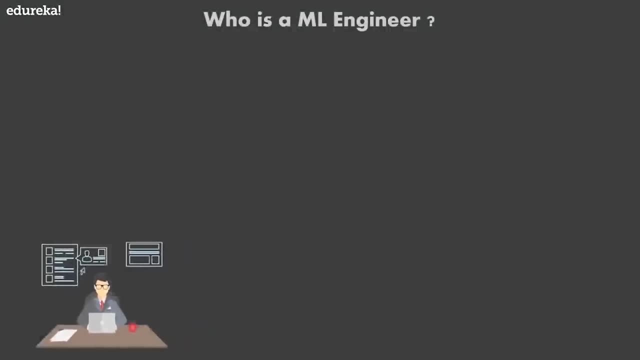 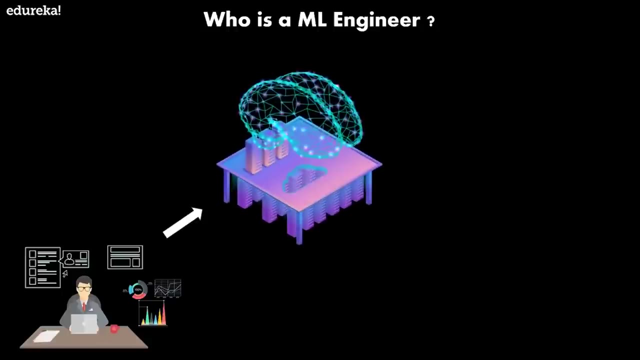 engineer while applying for a job. let's understand who exactly a machine learning engineer is. So machine learning engineers are sophisticated programmers who develop machines and systems that can learn and apply knowledge without specific direction. Artificial intelligence is the goal of a machine learning engineer. They are computer programmers, but their focus 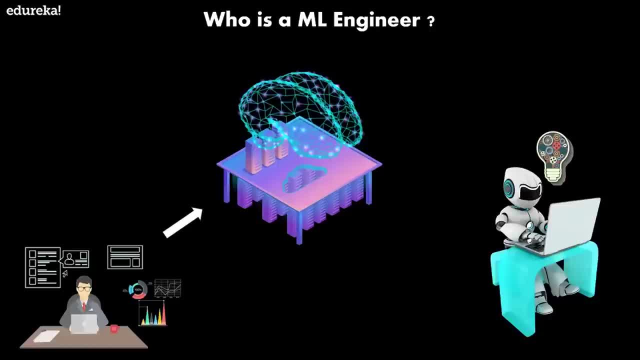 goes beyond specifically programming machines to perform specific tasks. They create programs that will enable machines to take actions without being specifically directed to perform those tasks. Now, if we have a look at the job trends of a machine learning engineer, So as you can see in, 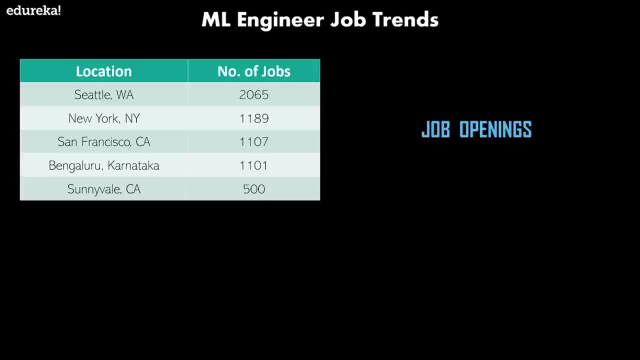 Seattle itself, we have 2000 jobs. in New York, we have 1100. in San Francisco, we have 1100. in Bengaluru, India, we have 1100, and then we have Sunnyvale, California, where we have 500 number of jobs. So as 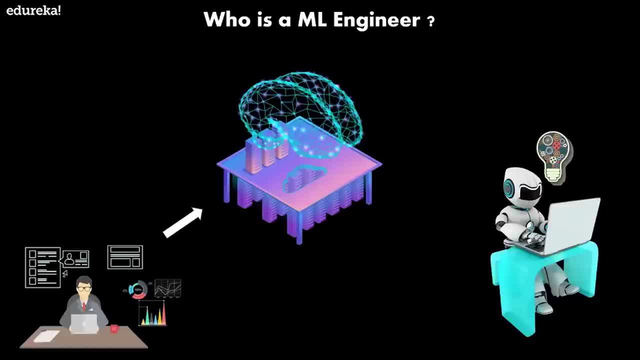 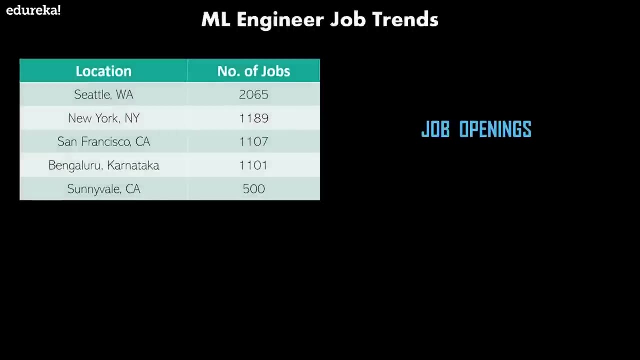 but their focus goes beyond specifically programming machines to perform specific tasks. they create programs that will enable machines to take actions without being specifically directed to perform those tasks. now, if we have a look at the job trends of a machine learning engineer, so as you can see, in seattle itself we have 2000 jobs. in new york we have 1100 in san francisco we 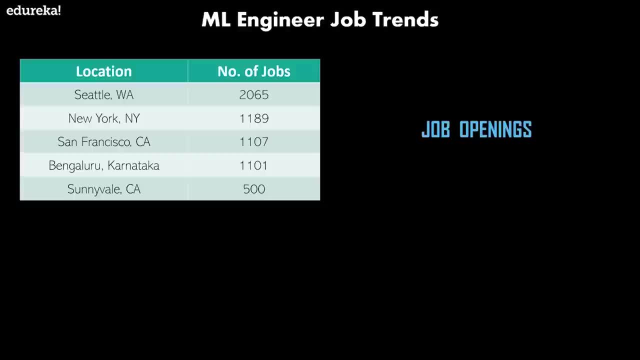 have 1100. in bengaluru, india, we have 1100, and then we have sunnyvale, california, where we have 500 number of jobs. so, as you can see, the number of jobs in the market is too much and probably with the emergence of 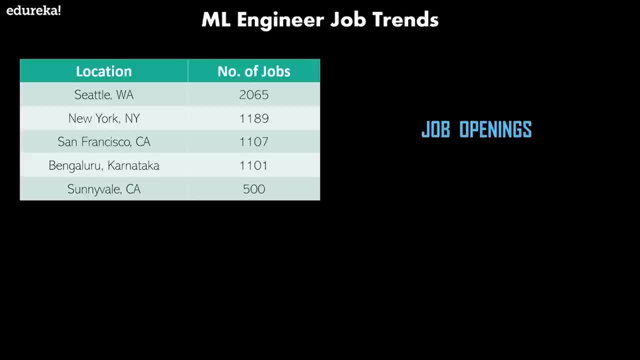 machine learning and artificial intelligence. this number is just going to get higher. now if we have a look at the job opening salary wise percentage, so we can see for the 90 000 per annum bracket we have 32.7 percentage and that's the maximum. so be assured that if you get a job as a machine, 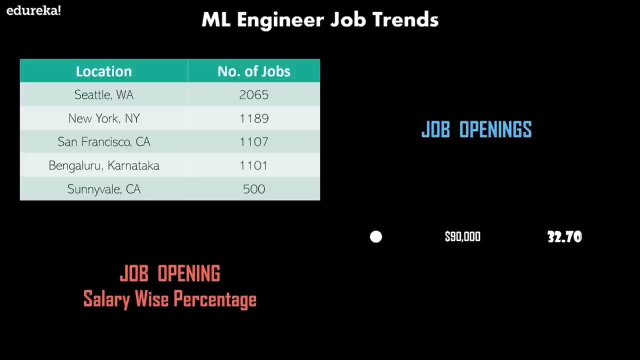 learning engineer, you'll probably get around 90 000 bucks a year. that's safe to say. now for the 110 000 per year, we have 25, 120 000, we have 20 almost. then we have 130 000, which are the senior. 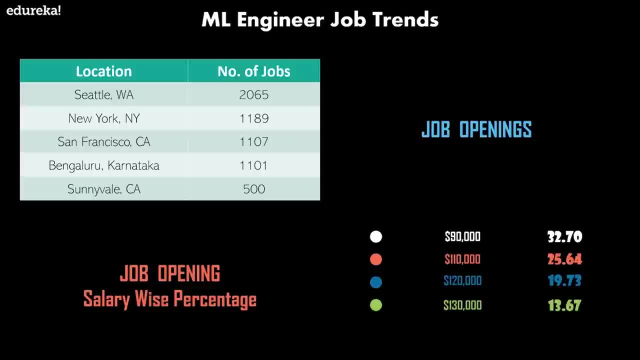 machine learning engineers, that's a 13.67. and finally we have the most senior machine learning engineer, or we have the data scientists here, which have the salary of 140 000 per annum, and the percentage for that one is really low. so, as you can see, there is a great opportunity for people. 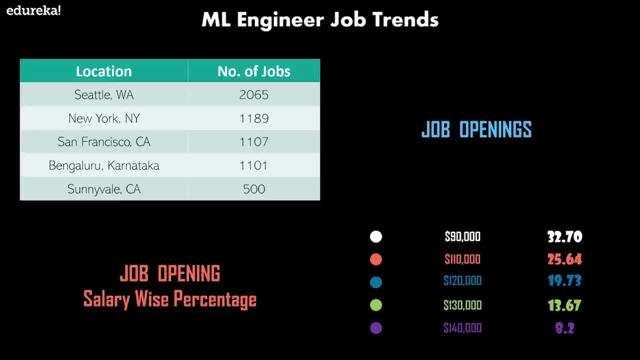 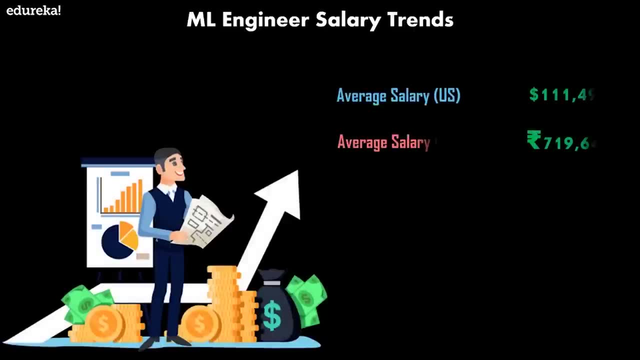 who are trying to go into the machine learning industry, and they are trying to go into the machine learning field and get started with it. so let's have a look at the machine learning engineer salary. so the average salary in the us is around 111 490 dollars and the average salary in india is around 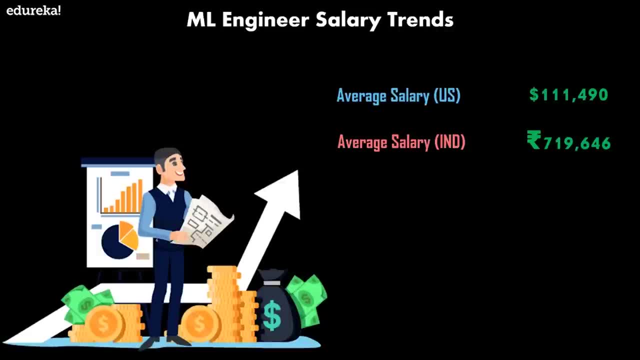 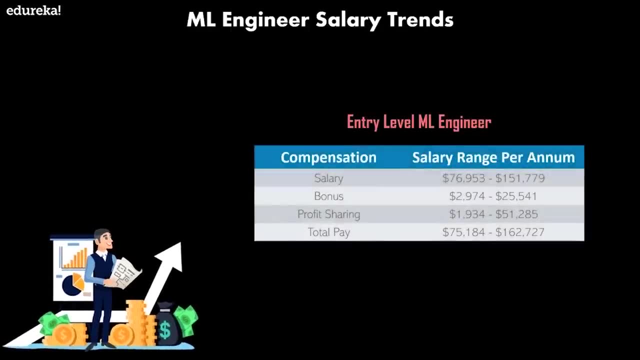 7 lakh 19 646 rupees. that's a very good average salary for any particular profession. so, moving forward, if we have a look at the salary of an entry-level machine learning engineer, so the salary is around 111 490 dollars and the average salary in india is around 7 lakh 19 646 rupees. 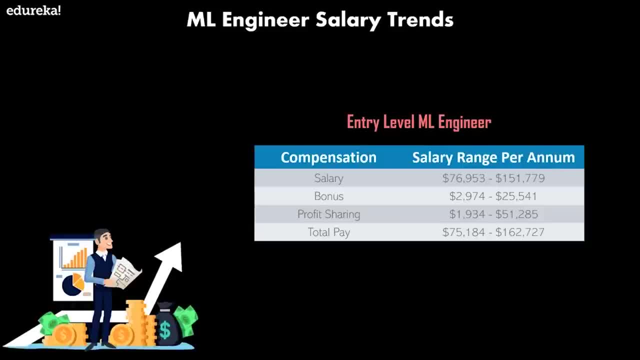 ranges from 76 000 or 77 000 to 151 000 per annum. that's a huge salary and if you talk about the bonus, here we have like three thousand dollars to twenty five thousand dollars, depending on the work you do and the project you are working on. let's talk about the profit sharing now. so it's 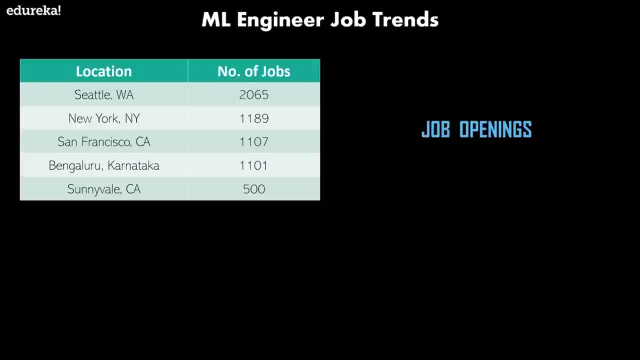 you can see, the number of jobs in the market is too much and probably with the emergence of machine learning and artificial intelligence, this number is just going to get higher. Now, if we have a look at the job opening salary wise percentage, so we can see, for the $90,000 per annum bracket we have, 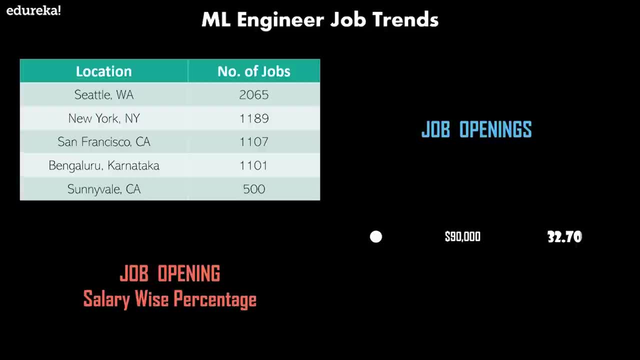 32.7 percentage and that's the maximum. So be assured that if you get a job as a machine learning engineer, you'll probably get around 90,000 bucks a year. that's safe to say. Now for the 110,000 dollars per year: we have 25 percent. 120,000 dollars, we have 20 percent, almost then we have 130,000. 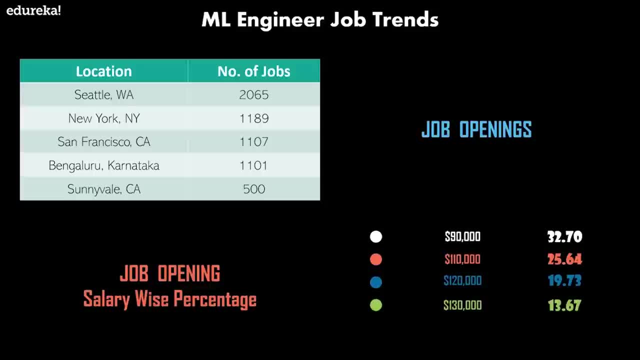 dollars, which are the senior machine learning engineers. that's a 13.67 percent. and finally, we have the most senior machine learning engineer, or we have the data scientists here, which have the salary of 140,000 dollars per annum, and the percentage for that one is really low. So, as you, 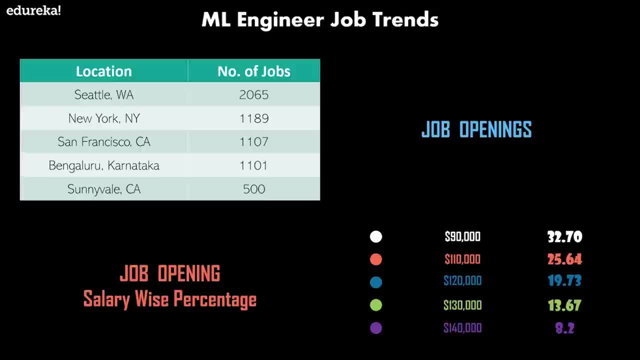 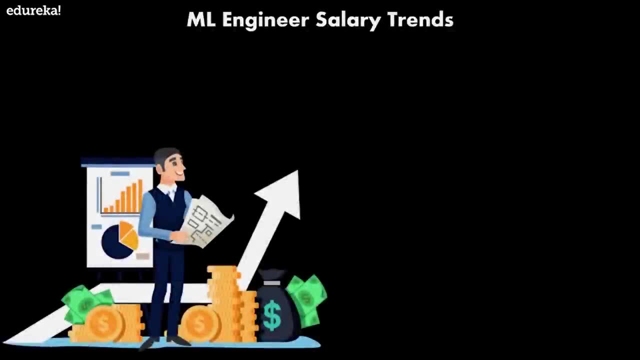 can see, there is a great opportunity for people who are trying to go into machine learning field and get started with it. So let's have a look at the machine learning engineer salary. So the average salary in the US is around 111,490 dollars and the average salary in India is around 7,19,646. 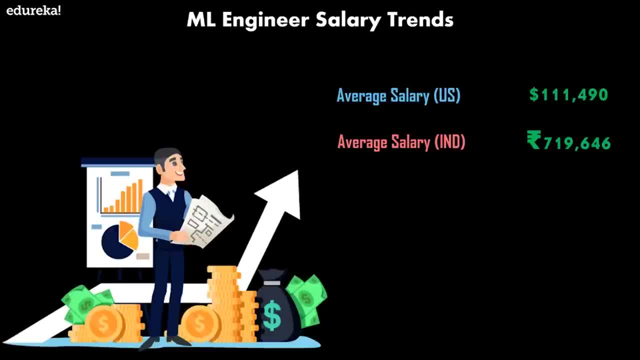 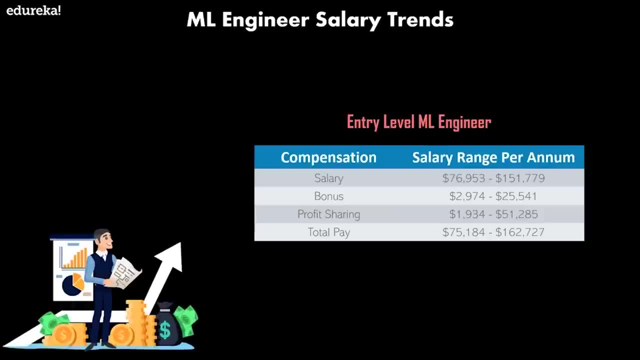 rupees. That's a very good average salary for any particular profession. So, moving forward, if we have a look at the salary of an entry-level machine learning engineer, So the salary ranges from 6,000 dollars or 77,000 dollars to 151,000 dollars per annum. That's a huge salary and if 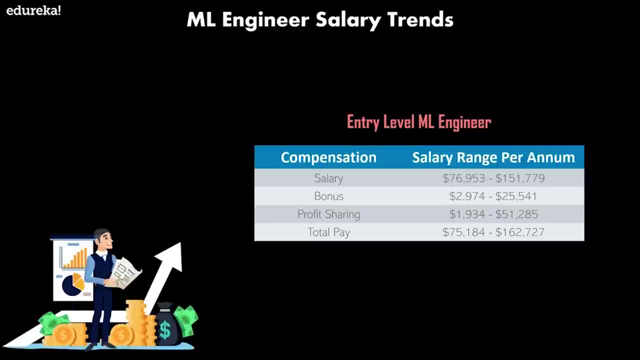 you talk about the bonus. here we have like 3,000 dollars to 25,000 dollars, depending on the work you do and the project you are working on. Let's talk about the profit sharing now. so it's around two thousand dollars to fifty thousand dollars. Now this again depends upon the project you are. 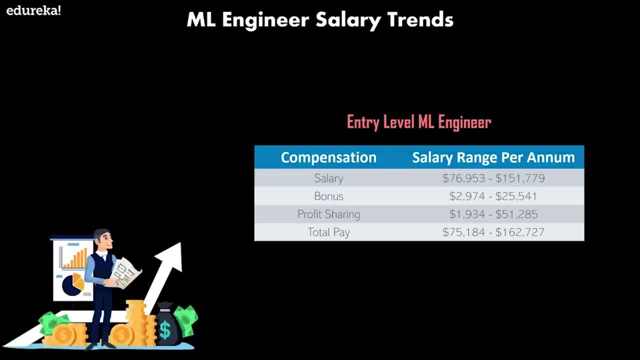 working, the company you are working for, and the percentage that they give to the engineer or the developer for that particular project. Now the total pay comes around 76,000 dollars, or 75,000 dollars to 162,000 dollars, and this is just for the entry-level machine learning engineer. Just. 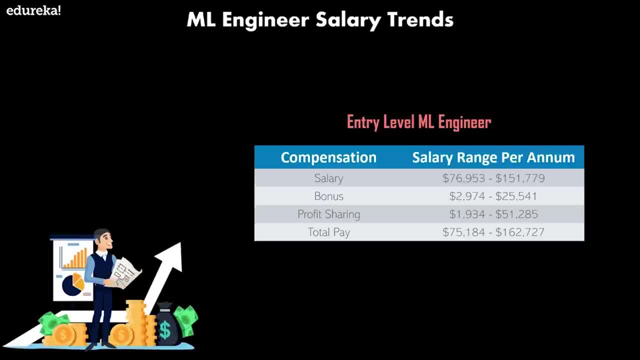 around two thousand dollars to fifty thousand dollars. now this again depends upon the project you are working, the company you are working for and the percentage that they give to the engineer or the developer for that particular project. now the total pay comes around seventy six thousand dollars or seventy five thousand dollars. two hundred and sixty two thousand. 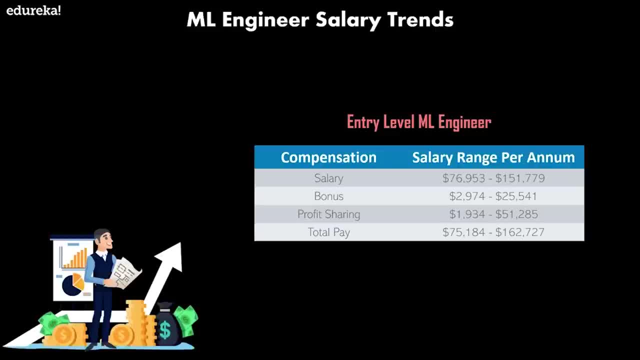 dollars, and this is just for the entry-level machine learning engineer. just imagine if you become an experienced machine learning engineer. your salary is going to go through the roof. so now that we have understood who exactly is a machine learning engineer, the various salary Trends, the job Trends in the market and how it's rising, let's understand what skills it 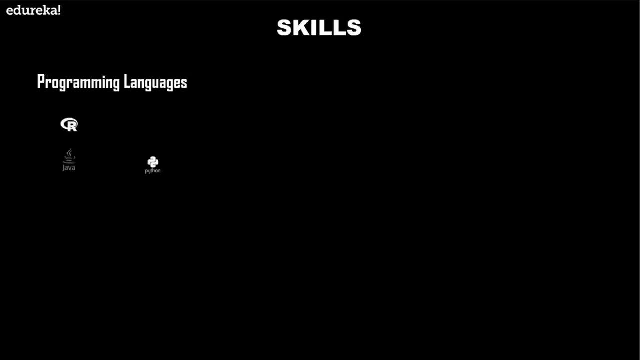 takes to become a machine learning engineer. so, first of all, we have programming languages. now, programming languages are a big deal when it comes to machine learning, because you don't just need to have proficiency in one language. you might require proficiency in python, Java, R or C++, because you 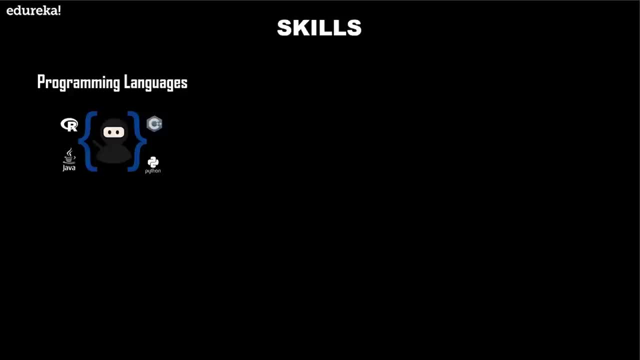 might be working in a Hadoop environment where you require Java programming to do the map, reduce codings and sometimes R is very great for visualization purposes and python, as you know, is one when it comes to machine learning. now, next skill that particular individual needs is calculus, and 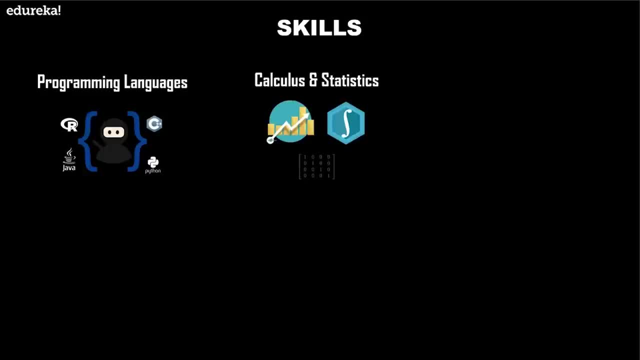 statistics. so a lot of machine learning algorithms are mostly maths and statistics so, and a lot of statistic is required. majorly, the matrix, multiplication and all. so good understanding of calculus as well as statistic is required now. next we have signal processing. now, advanced signal processing is something that will give you an upper edge over other machine learning engineers. 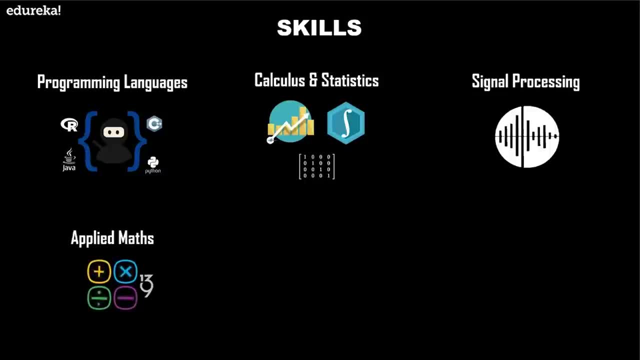 if you are applying for a job now, the next skill we have is applied maths. as I mentioned earlier, many of the machine learning algorithms here are purely mathematical formulas, so a good understanding of maths and how the algorithm works will take you far ahead now. next on our list we have neural networks. now neural. 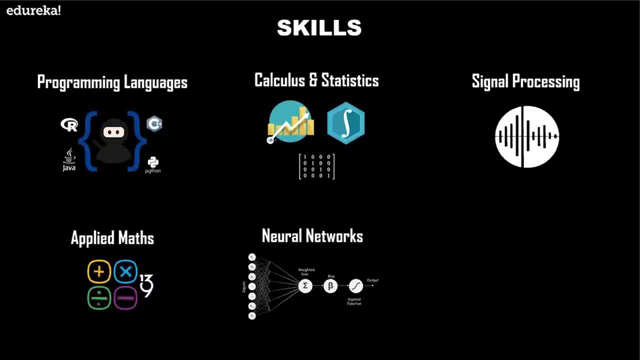 networks are something that has been emerging quite popularly in the recent years and, due to its efficiency and the extent to which it can work and get the results as soon as possible, neural networks are a must for a machine learning engineer. now moving forward, we have language processing, so a lot of 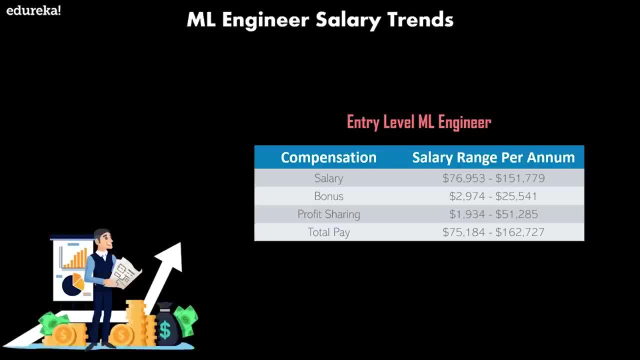 imagine if you become an experienced machine learning engineer. your salary is going to go through the roof. So now that we have understood who exactly is a machine learning engineer, the various salary trends, the job trends in the market and how it's rising, let's understand what skills 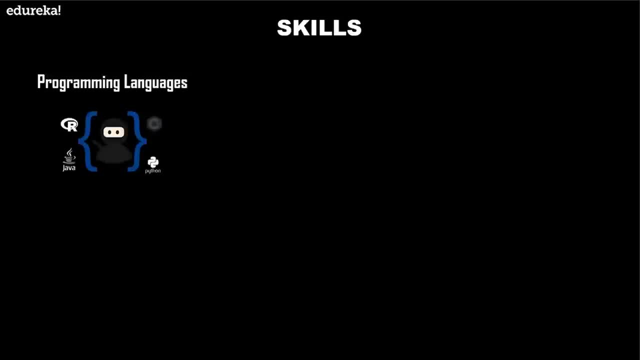 you need to become a machine learning engineer. So, first of all, we have programming languages. now, Programming languages are a big deal when it comes to machine learning, because you don't just need to have proficiency in one language. You might require proficiency in Python, Java, R or C++, because you 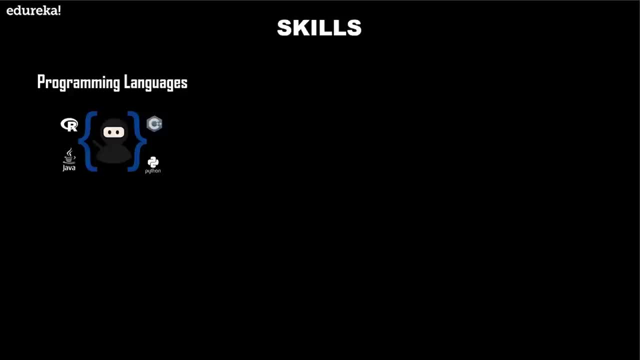 might be working in a Hadoop environment where you require Java programming to do the MapReduce codings and sometimes R is very great for visualization purposes and Python, as you know, is for machine learning. Now, next skill that a particular individual needs is calculus and statistics, So a lot of machine learning algorithms are mostly maths and statistics. so, and a lot of 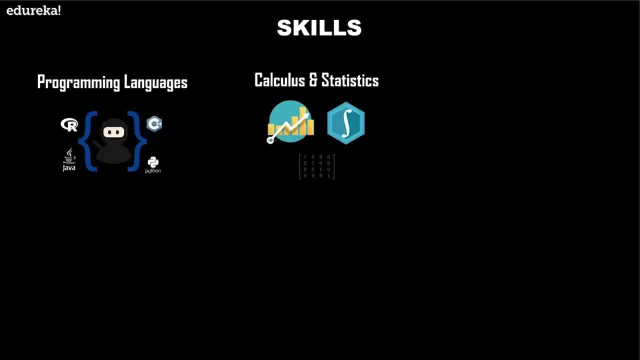 statistic is required, majorly: the matrix, multiplication and all. So good understanding of calculus as well as statistic is required Now. next we have signal processing. Now, advanced signal processing is something that will give you an upper edge over other machine learning engineers if you are applying for a job anywhere. 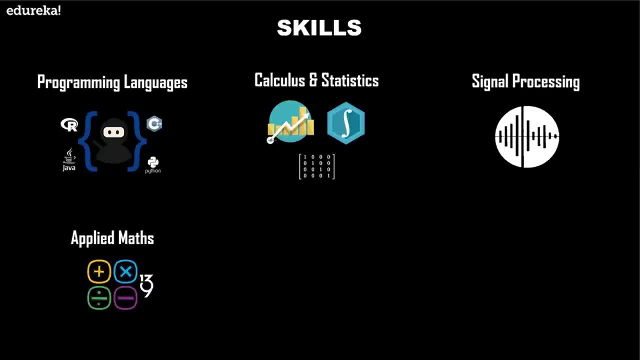 So the next skill we have is applied maths. As I mentioned earlier, many of the machine learning algorithms here are purely mathematical formulas, So a good understanding of maths and how the algorithm works will take you far ahead. Now, next on our list, we have neural networks. Now neural. 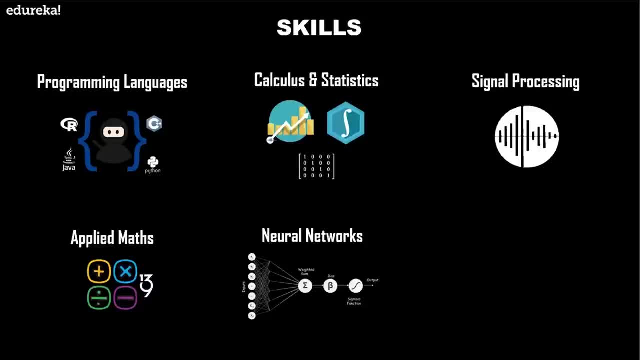 networks are something that has been emerging quite popularly in the recent years and, due to its efficiency and the extent to which it can work and get the results as soon as possible, neural networks are a must for a learning engineer. now moving forward, we have language processing, so a lot of 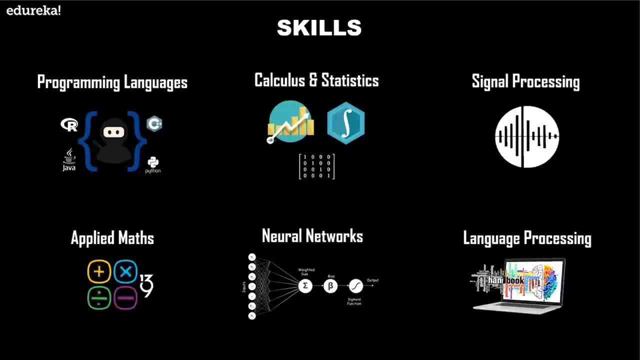 times, machine learning engineers have to deal with text data, the voice data, as well as video data. now, processing any kind of language, audio or the video is something that a machine learning engineer has to do on a daily basis, so one needs to be proficient in this area also. now, these were only some of the few. 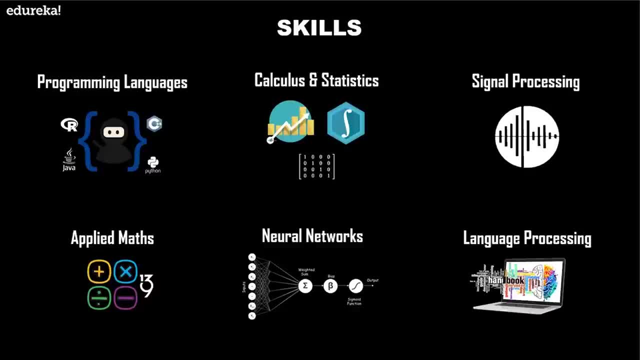 times, machine learning engineers have to deal with text data, the voice data, as well as video data. now, processing any kind of language, audio or the video is something that a machine learning engineer has to do on a daily basis, so one needs to be proficient in this area also. now, these were only some of the 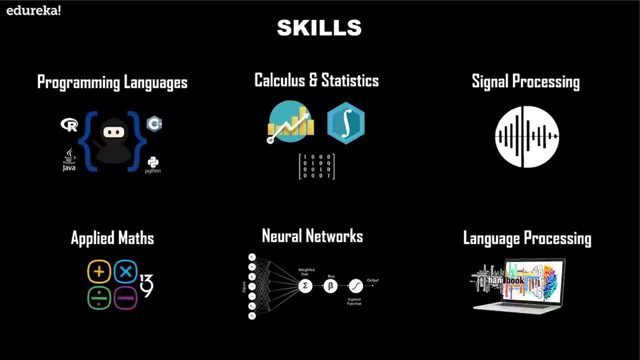 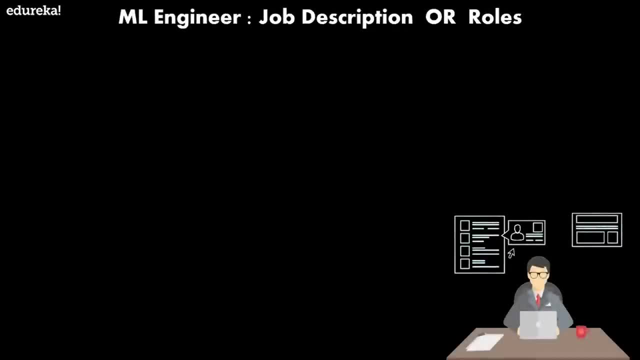 few skills which are absolutely necessary, I would say, for any machine learning engineer. so let's now discuss the job description, or the roles and responsibilities of a particular machine learning engineer. now, depending on their level of expertise, machine learning engineers may have to study and transform data science prototypes. they need to design machine learning systems. they also. 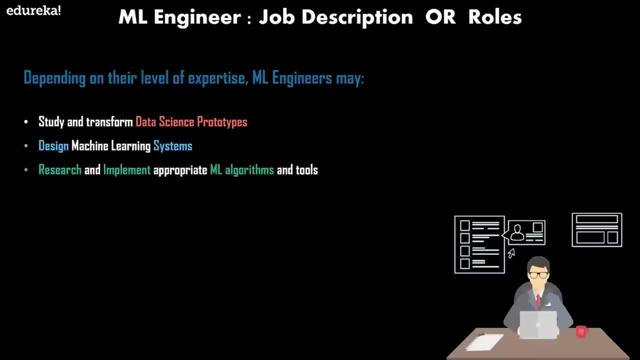 need to research and implement appropriate machine learning algorithms and tools, as it's a very important part of the job. they need to develop new machine learning application according to the industry requirements. they need to select the appropriate data sets and the data representation methods, because if there is a slight deviation in the 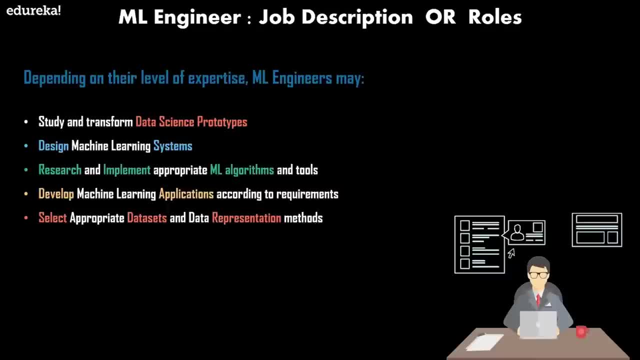 data set and the data representation that's going to affect the model a lot. they need to run machine learning tests and experiments. they need to perform statistical analysis and fine tuning using the test results. so sometimes people ask what exactly is the difference between a data analyst and a machine learning engineer? so so statistical analysis is just a small part of a machine learning. 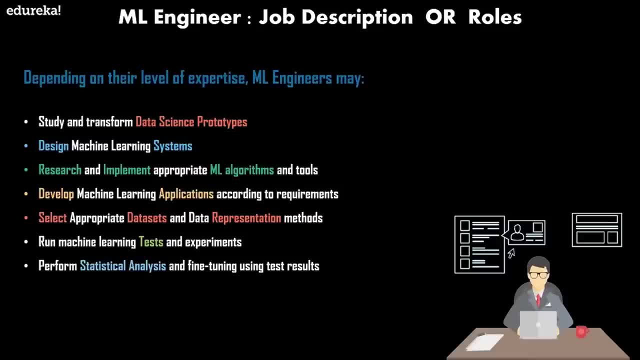 engineer's job, whereas it is a major part- or it probably covers a large part- of a data analyst job rather than a machine learning engineer's job. so machine learning engineers might need to train and retrain the systems whenever necessary, and they also need to extend the existing machine learning libraries and 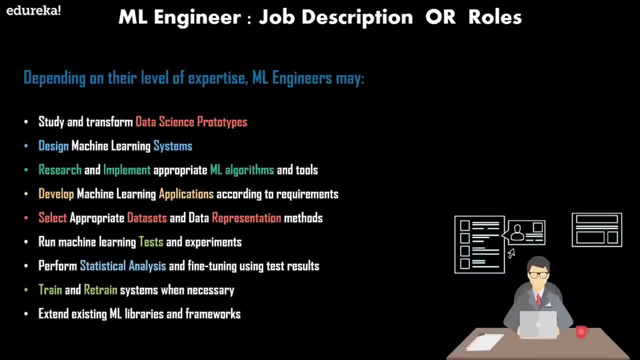 frameworks to their full potential so that they could make the model work superbly. and finally, they need to keep abreast of the developments in the field, needless to say that any machine learning engineer or any particular individual has to stay updated to the technologies that are coming in the market, and every. 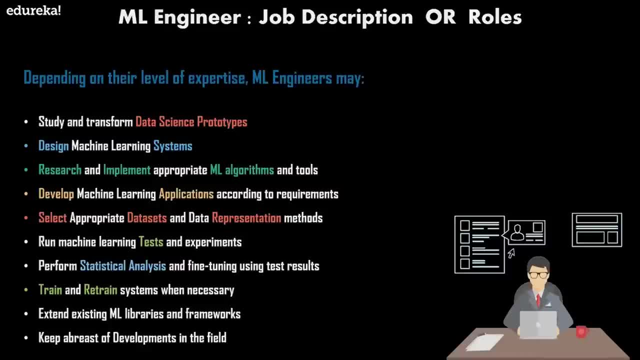 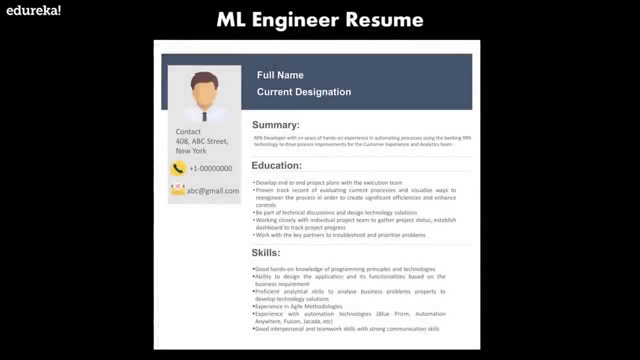 now and then a new technology arises which will overthrow the older one, so you need to be up to date. now coming to the resume part of a machine learning engineer. so any resume of a particular machine learning engineers should consist like clear career objective: the skills which a particular 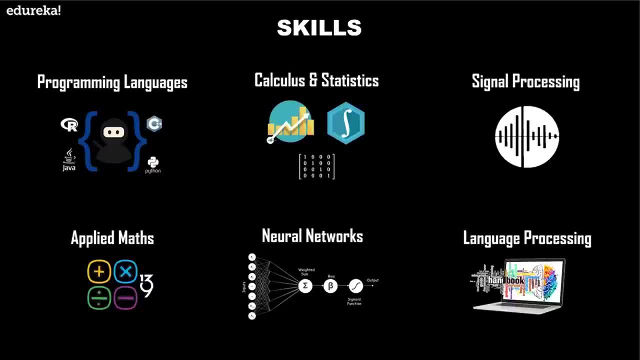 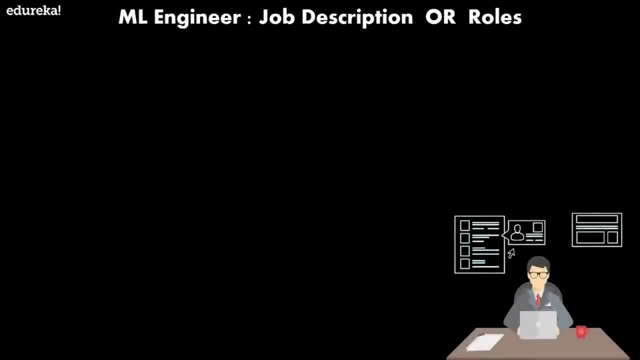 skills which are absolutely necessary, I would say, for any machine learning engineer. so let's now discuss the job description, or the roles and responsibilities of a particular machine learning engineer. now, depending on their level of expertise, machine learning engineers may have to study and transform data science prototypes. they need to design machine learning systems. 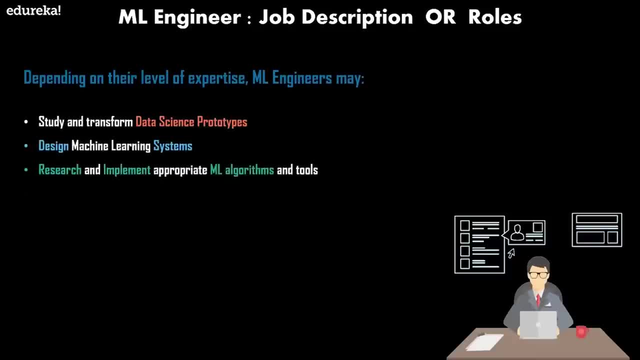 they also need to research and implement appropriate machine learning algorithms and tools, as it's a very important part of the job. they need to develop new machine learning application according to the industry requirements and they need to select the appropriate data sets and the data representation methods, because if there is a slight deviation in the data set and the data, 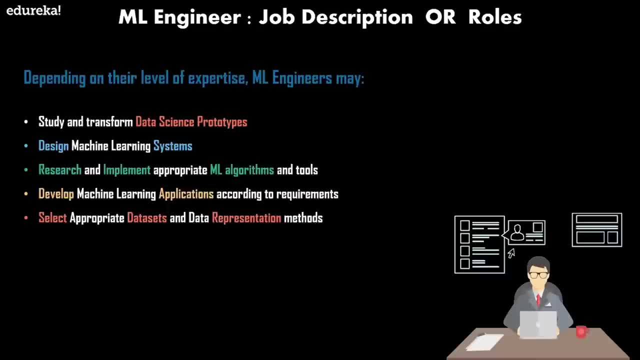 representation. that's going to affect the model a lot. they need to run machine learning tests and experiments. they need to perform statistical analysis and fine-tuning using the test results. so sometimes people ask what exactly is the difference between a data analyst and a machine learning engineer? 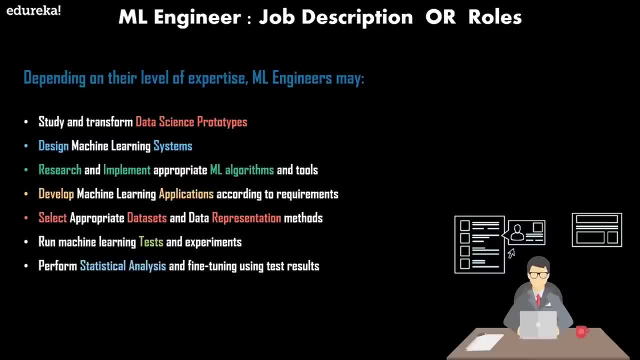 so. so statistical analysis is just a small part of machine learning engineers job, whereas it is a major part- or it probably covers a large part- of a data analyst job rather than a machine learning engineer's job. so Machine Learning engineers might need to train and retrain the systems whenever necessary, and they also need to 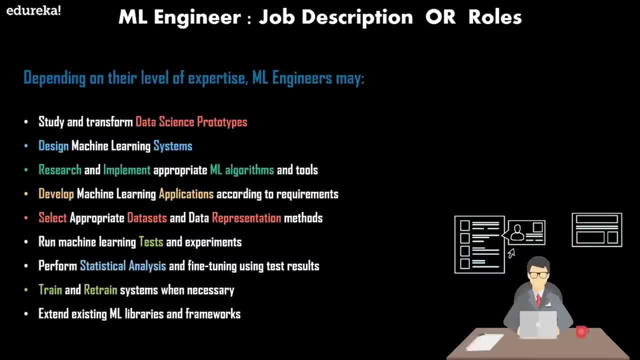 extend the existing machine running libraries and frameworks to their full potential so that they could make the model work superbly. and finally, they need to keep abreast of the developments in the field, needless to say that any machine learning engine or any particular individual has to stay. 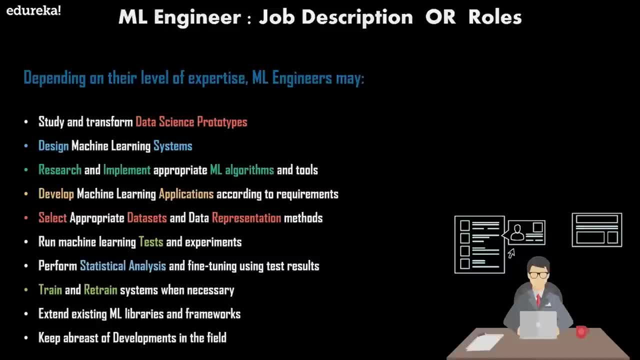 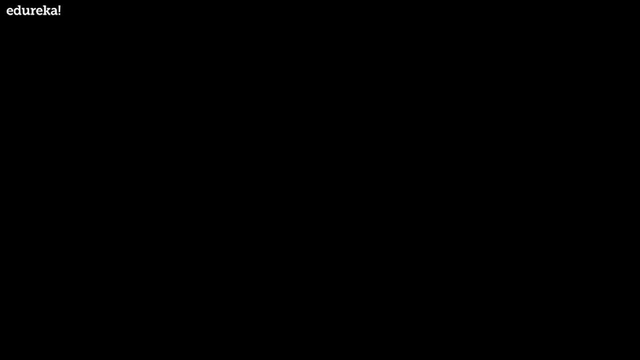 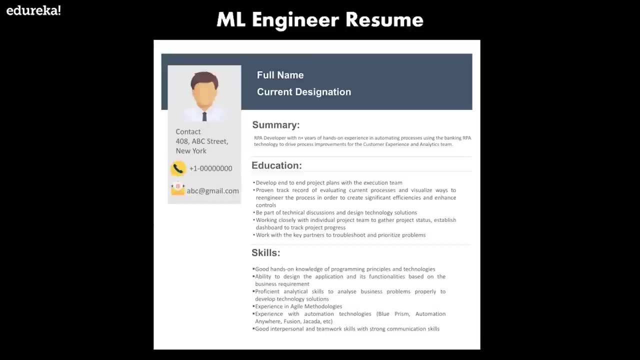 updated to the technologies that are coming in the market, and every now and then a new technology arises which will overthrow the older one, so you need to be up to date. now coming to the resume- part of a machine learning engineer. so any resume of a particular machine learning engineers should consist like: 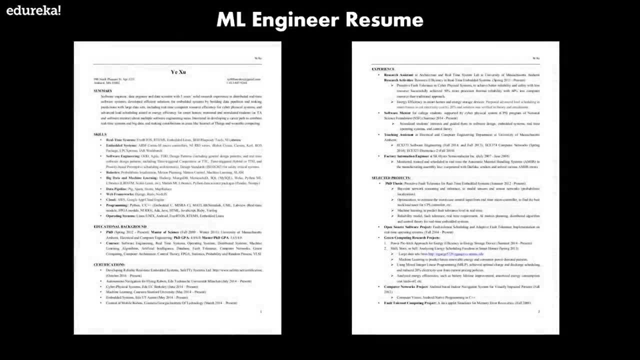 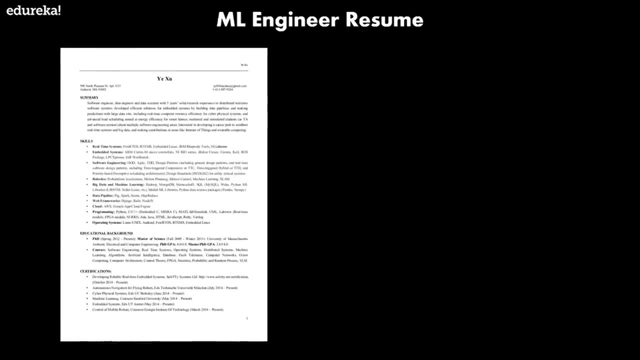 clear career objective, the skills which a particular individual possesses, the educational qualification, certain certification, the past experience- if you are an experienced machine learning engineer, the projects which you have worked on and that's it. so let's have a look at the various elements that are required in a machine learning engineers resume. so, first of all, you need to have 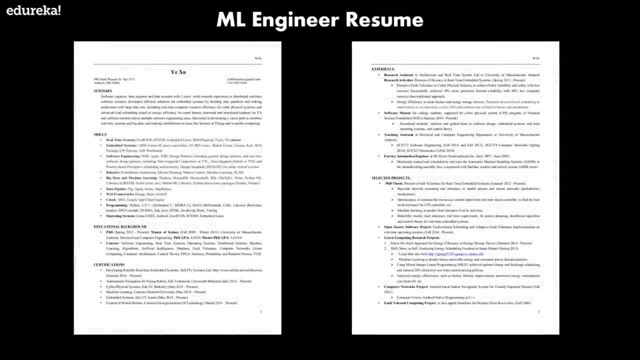 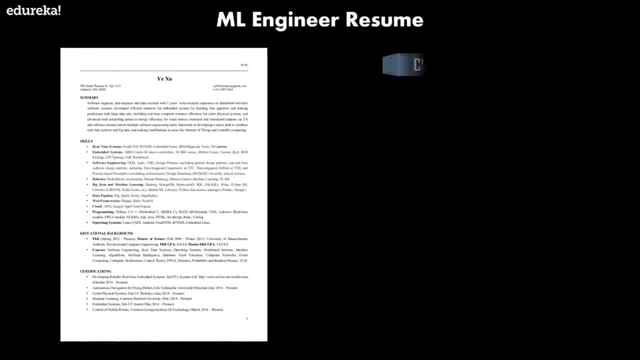 individual possesses the educational qualification, certain certification, the past experience- if you are a machine learning engineer, the projects which you have worked on and that's it. so let's have a look at the various elements that are required in a machine learning engineer's resume. so first of all, you need 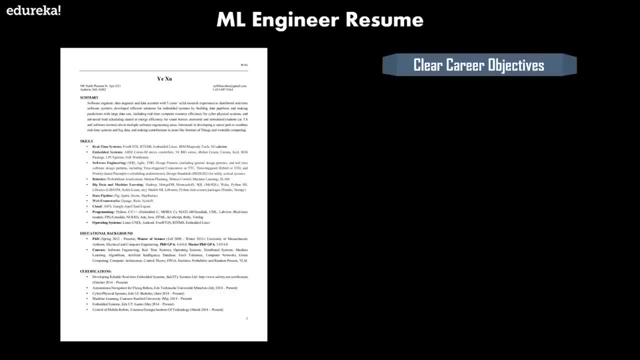 to have a clear career objective. so here you need not stretch it too much and keep it as precise as possible. so next we have the skills required, and these skills can be technical as well as non-technical. so let's have a look at the various technicals and the non-technical skills out here. so, starting with, 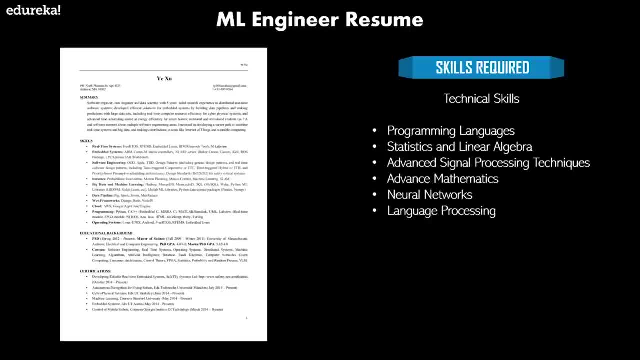 technical skills. first of all, we have programming languages, as in R, Java, Python and C++, but the first and the foremost requirement is to have a good grip on any programming languages, preferably python, as it is easy to learn and its applications are wider than any other language. now it is 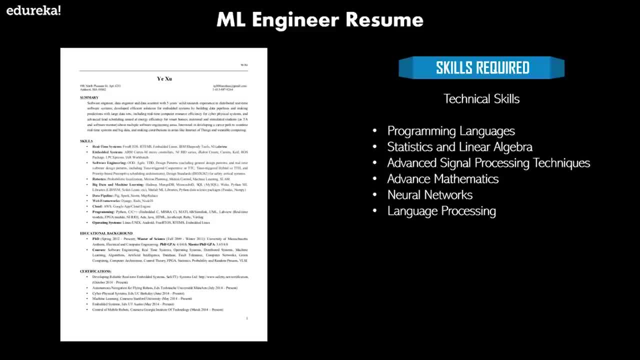 important to have a good understanding of topics like data structures, memory management and classes. although python is a very good language, it alone cannot help you, so you will probably have to learn all these languages like C++, R, python, Java, and also work on MapReduce at some point of time. the next on our list: we have calculus. 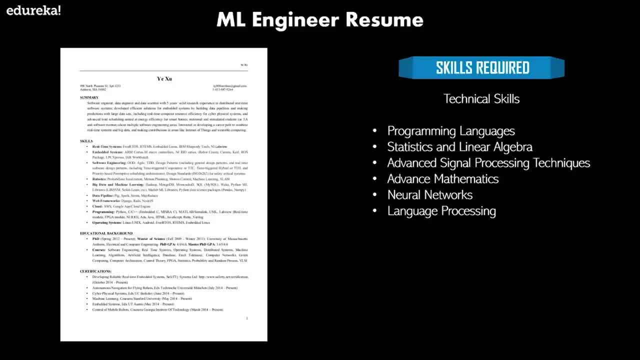 and linear algebra and statistics. so you'll need to be intimately familiar with matrices, the vectors and the matrix multiplication. so statistics is going to come up a lot and at least make sure you are familiar with Gaussian distribution, means, standard deviations and much more. so you also need to have a firm understanding of probability and stats to 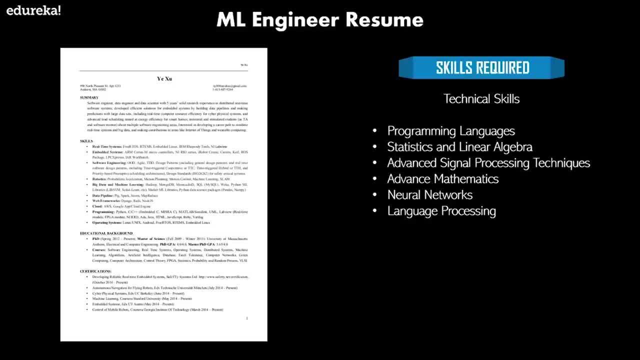 understand the machine learning models now. next, as I mentioned earlier, it's signal processing techniques. so feature extraction is one of the most important parts of machine learning. different types of problems need various solutions, so you may be able to utilize the really cool advanced signal processing algorithms such as wavelets, chairlets, curvelets and the bandlets. so try to. 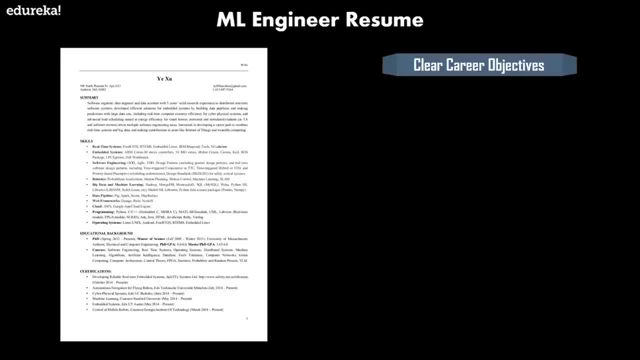 a clear career objective. so here you need not stretch it too much and keep it as precise as possible. so next we have the skills required, and these skills can be technical as well as non-technical. so let's have a look at the various technicals and the non-technical skills out here. so 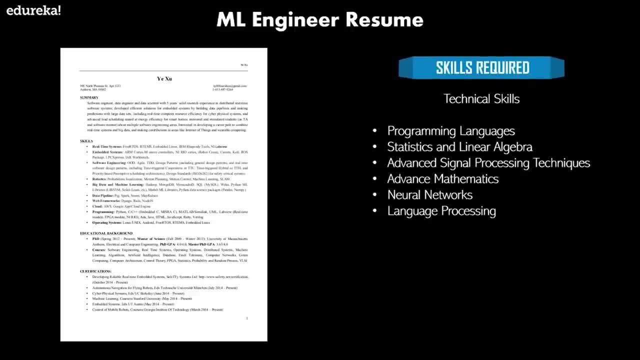 starting with the technical skills. first of all, we have programming languages, as in our Java, Python and C++, but the force in the foremost requirement is to have a good grip on any programming languages, preferably Python, as it is easy to learn and its applications are wider than any other language. now it is important to 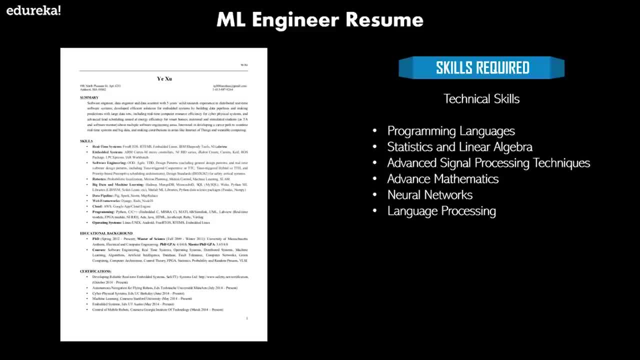 have a good understanding of topics like data structures, memory management and classes. all the Python is a very good language. it every other language, so you may need to have a good context to address. your alone cannot help you, so you will probably have to learn all these languages, like c plus plus r, python, java and also work on map. 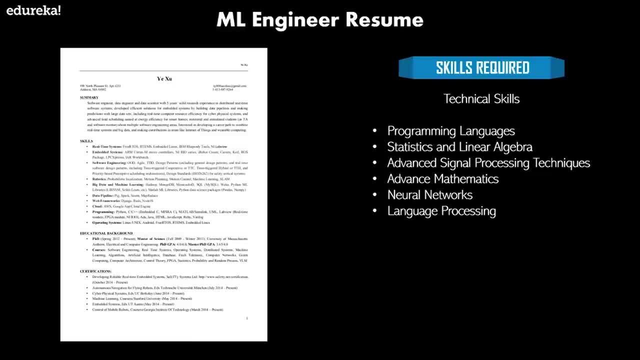 reduce at some point of time now. next on our list we have calculus and linear algebra and statistics, so you'll need to be intimately familiar with matrices, the vectors and the matrix multiplication. so statistics is going to come up a lot, and at least make sure you are familiar with gaussian distribution. 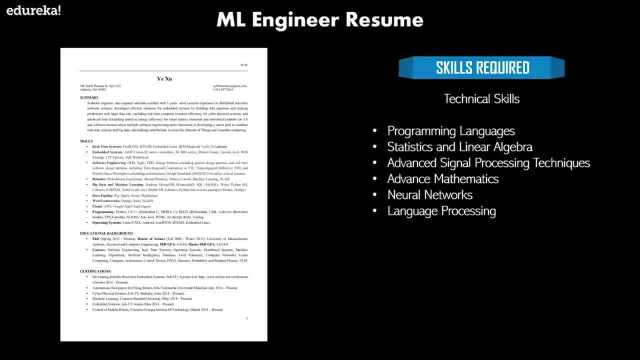 mean standard deviations and much more. so you also need to have a firm understanding of probability and stats to understand the machine learning models. now next, as i mentioned earlier, it's signal processing techniques. so feature extraction is one of the most important parts of machine learning. different types of problems need various 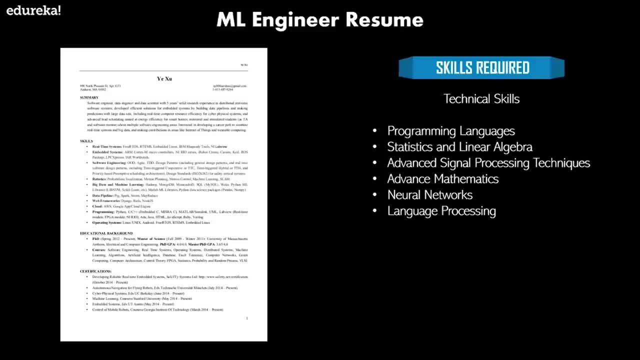 solutions so you may be able to utilize the really cool advanced signal processing algorithms such as wavelets, chairlets, curvelets and the bandlets. so try to learn about the time frequency analysis and try to apply it to your problems, as it gives you an upper edge over other. 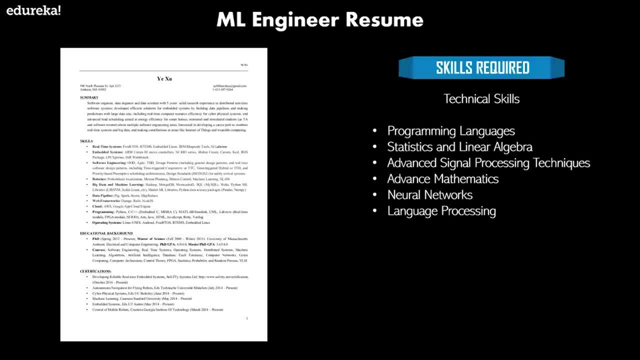 machine learning engineers. so just go for it now. next we have mathematics and a lot of machine learning techniques out. there are just fancy types of function approximation. having a firm understanding of algorithm theory and knowing how the algorithm works is really necessary, and understanding subjects like gradient descent. 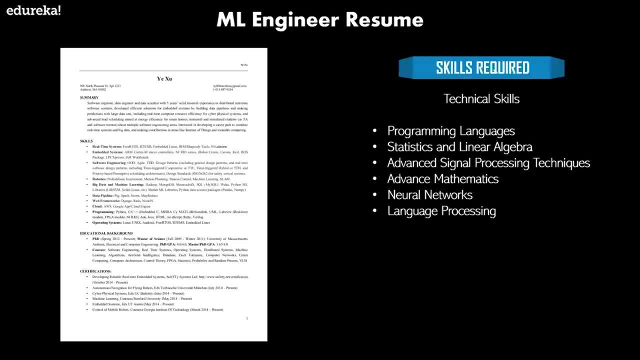 learn about the time frequency analysis and try to apply it to your problems, as it gives you an upper edge over other machine learning engineers. so just go for it. the next we have mathematics and a lot of machine learning techniques out. there are just fancy types of function approximation: having a firm understanding. 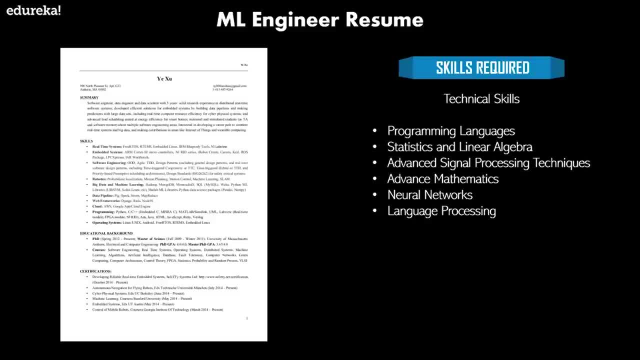 of algorithm theory and knowing how the algorithm works is really necessary, and understanding subjects like gradient descent, convex optimization, quadratic programming and partial differentiation will help a lot. the neural networks, as I was talking earlier. so we need machine learning for tasks that are too complex for humans, to quote. 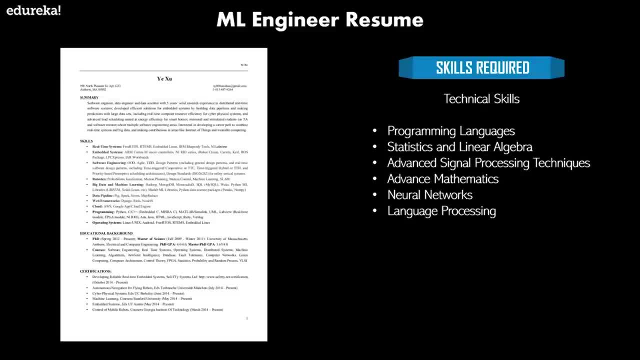 directly, so that is, the tasks that are so complex that it is impractical. the neural networks are a class of models within the general machine learning literature. they are specific set of algorithms that have revolutionized machine learning. deep neural networks have proven to work quite well and neural networks are themselves general function approximations, which is why they can be applied to. 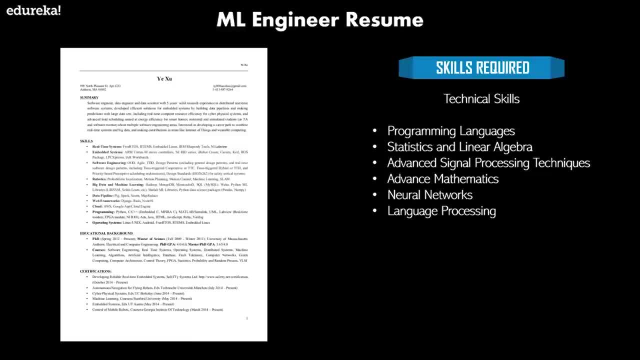 almost any machine learning problem out there and they help a lot about learning a complex mapping from the input to the output space. so next we have language processing, since natural language processing combines two of the major areas of work, that are, linguistic and computer science, and chances are at some point you are going to 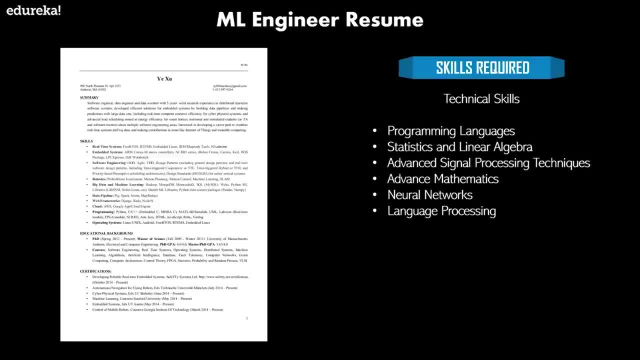 work with either text or audio or the video, so it's necessary to have a control over libraries like gensim nltk and techniques like word to wet, sentimental analysis and text summarization. now, voice and audio analysis involves extracting useful information from the audio signals themselves. being well versed in maths and concept like fourier transformation will get you far in this one. 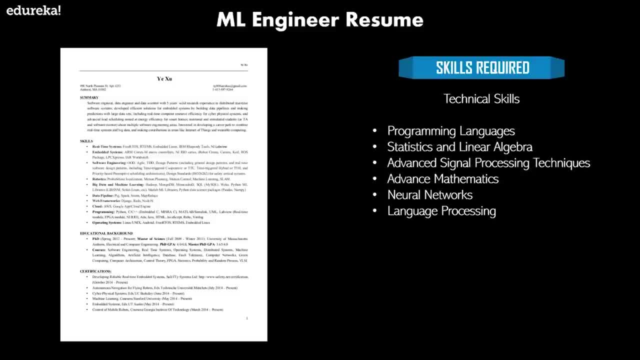 now, these were the technical skills that are required, but be assured that there are a lot of non-technical skills also that are required to land a good job in a machine learning industry. so first of all, you need to have an industry knowledge. so the most successful machine learning projects 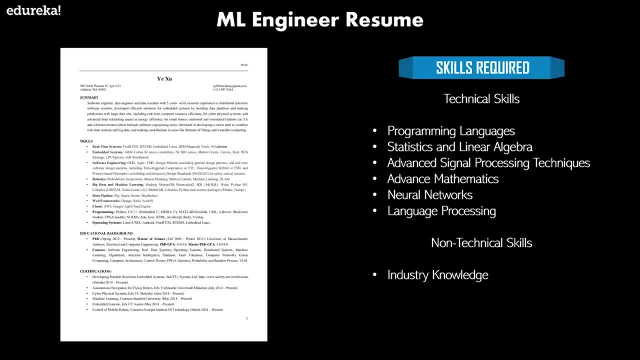 out, there are going to be those that address real pain points, don't you agree? so, whichever industry you are working for, you should know how that is going to work and how you are going to be able to work in the industry. you should know how that is going to work and how you are going to be able to work in the industry. 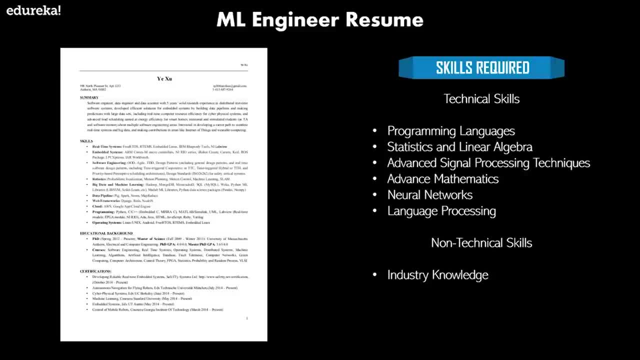 works and what will be beneficial for the industry now, if a machine learning engineer does not have business acumen and the know-how of the elements that make up a successful business model, all those technical skills cannot be channeled productively. you won't be able to. 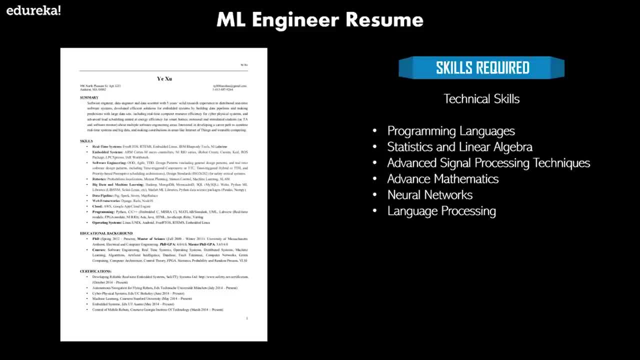 convex optimization, quadratic programming and partial differentiation help a lot. the neural networks, as i was talking earlier. so we need machine learning for tasks that are too complex for humans to code directly, so that is, the tasks that are so complex that it is impractical. the neural networks are a class of models within the general machine learning. 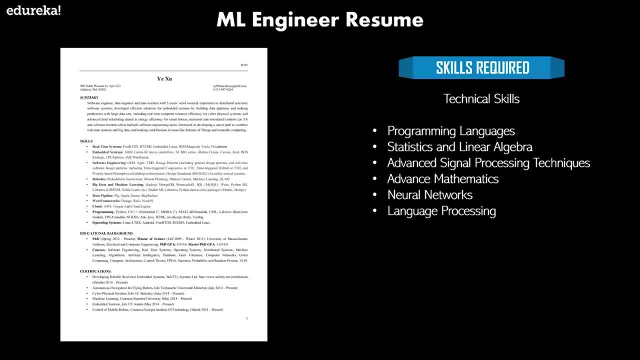 literature. they are specific set of algorithms that have revolutionized machine learning. deep neural networks have proven to work quite well and neural networks are themselves general function approximations, which is why they can be applied to almost any machine learning problem out there and they help a lot about learning a complex mapping from the input to the output space. 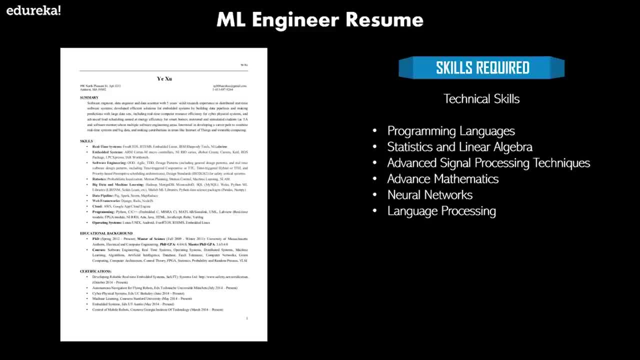 now. next we have language processing, since natural language processing combines two of the major areas of work, that are, linguistic and computer science, and chances are at some point you are going to work with either text or audio or the video, so it's necessary to have a control over 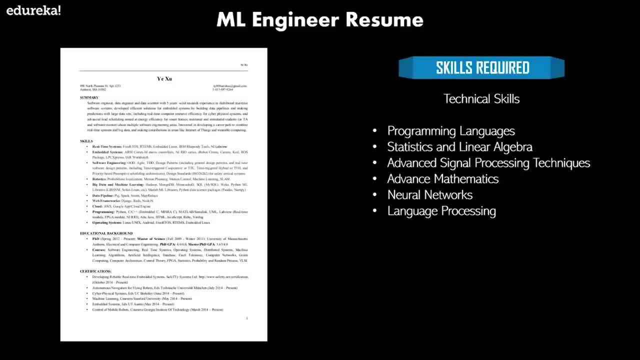 libraries like gen, sim, nltk, and techniques like and text summarization. now, voice and audio analysis involves extracting useful information from the audio signals themselves. being well versed in maths and concept like fourier transformation will get you far in this one. now, these were the technical skills that are required, but be assured, 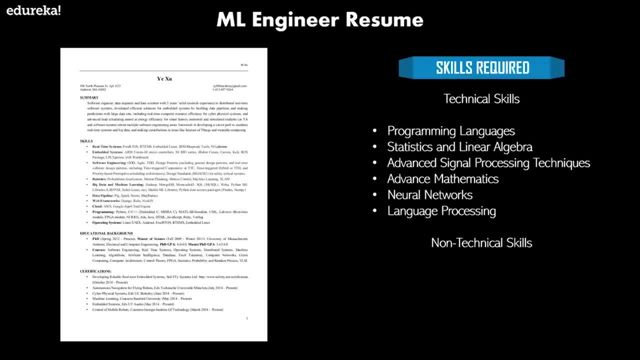 that there are a lot of non-technical skills also that are required to land a good job in a machine learning industry. so first of all you need to have an industry knowledge. so the most successful machine learning projects out there are going to be those that address real pain. 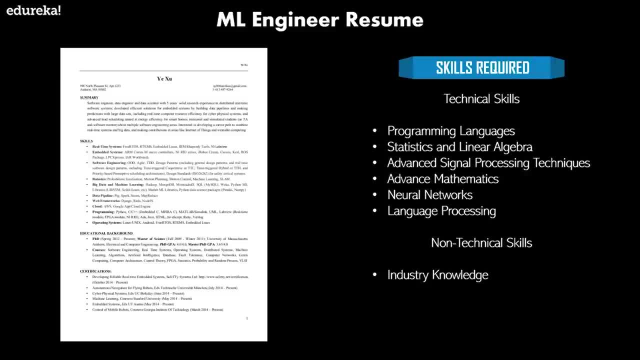 points, don't you agree? so whichever industry you are working for, you should know how that industry works and what will be beneficial for the industry now if a machine learning engineer does not have business acumen and the know-how of the elements that make up a successful business model? all those? 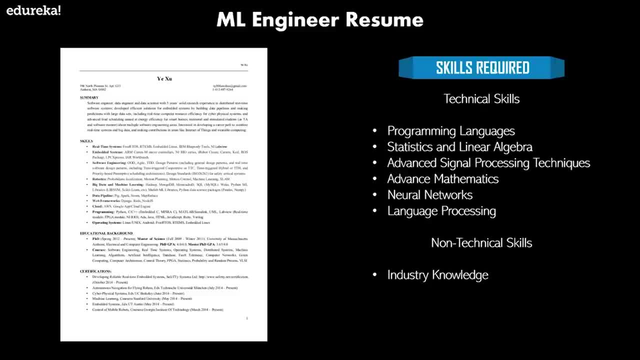 technical skills cannot be channeled productively, you won't be able to discern the problems and the potential challenges that need solving for the business to sustain itself. so you need to have a strong machine learning engineer and grow now. next in our list, we have effective communication and 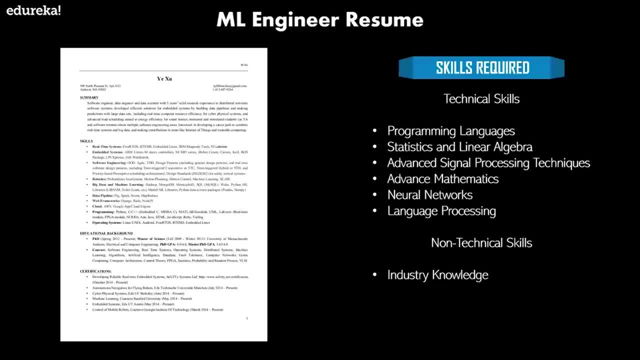 discern the problems and the potential challenges that need solving for the business to sustain and grow. now next in our list we have effective communication, and now this is one of the most important parts in any job requirements, so you'll need to explain machine learning concepts to people with little to no expertise in the field. the chances are you will need to work with 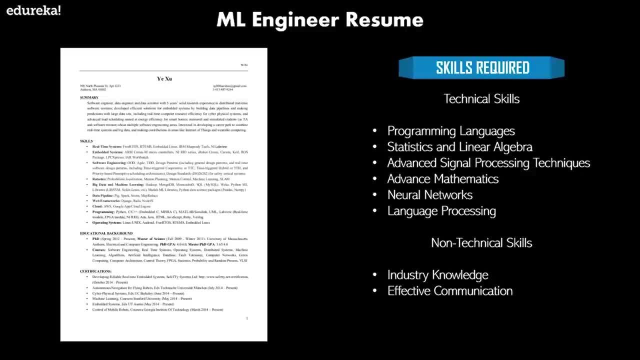 a team of engineers, as well as many other teams like marketing and the sales team, so communication is going to make all of this much easier. companies searching for a strong machine learning engineer are looking for someone who can clearly and fluently translate their technical findings to a non-technical team. now rapid prototyping is another skill which is very much required. 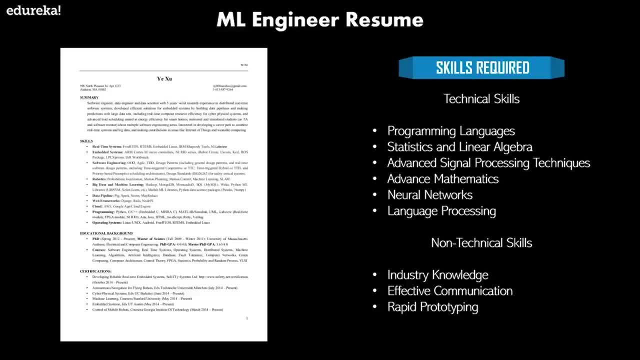 for any machine learning engineer, so iterating on ideas as quickly as possible is mandatory for finding the one that works in machine learning. this applies to everything from picking the right model to working on projects such as a, be testing and much more. now you need to do a group of techniques used to quickly fabricate a. 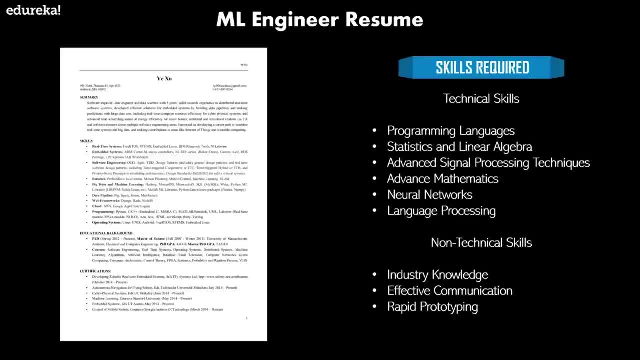 scale model of a physical part or assembly using the three-dimensional computer area design, which is the CAD data now coming to, the final skills which will be required for any machine learning engineer is to keep updated. now you must stay updated with any upcoming changes. every month, new neural network models come out that outperform the 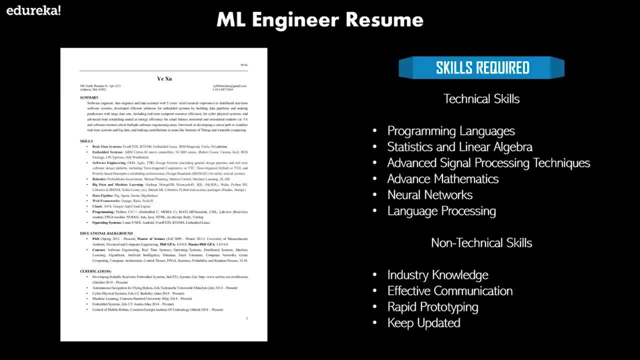 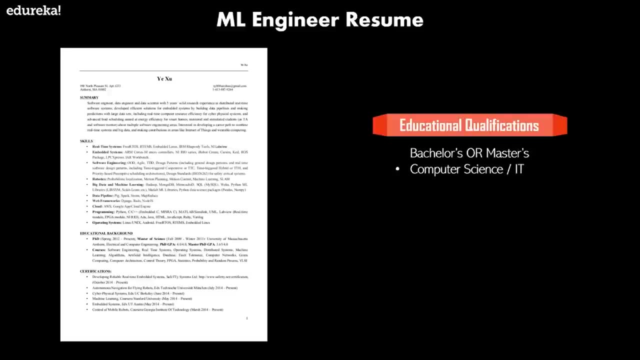 previous architecture. it also means being aware of the news regarding the development of the tools, theory and algorithms through research papers, blogs, conference videos and much more. now, another part of any machine learning engineers resume is the educational qualification, so a bachelor's or a master's degree in computer science or IT, economics, statistics or even 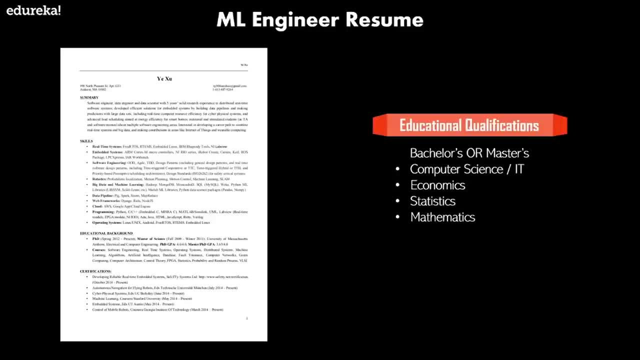 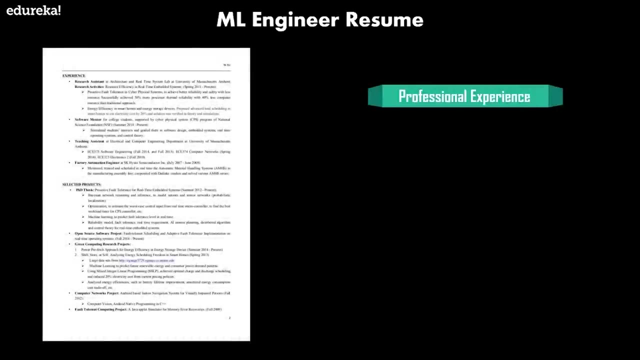 mathematics can help you land a job in machine learning. plus, if you are an experienced machine learning engineer, so probably some standard company certifications will help you a lot by landing a good job in machine learning. and finally, coming to the professional experience: you need to have experience in computer science. 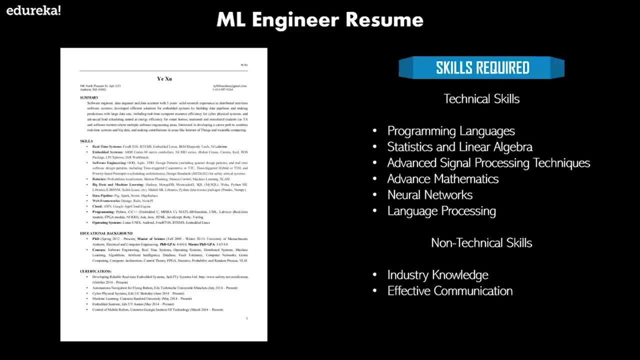 now. this is one of the most important parts in any job requirements, so you'll need to explain machine learning concepts to people with little to no expertise in the field. the chances are you will need to work with a team of engineers, as well as many other teams like marketing and the sales. 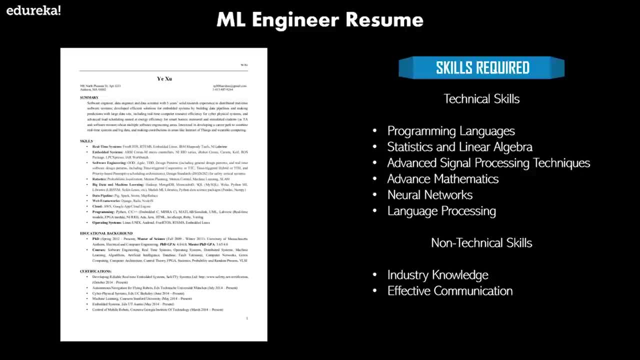 team. so communication is going to make all of this much easier. companies searching for a strong machine learning engineer are looking for someone who can clearly and fluently translate the technical findings to a non technical team. now, rapid prototyping is another skill which is very much required for any machine learning engineer, so iterating on ideas as quickly as possible is. 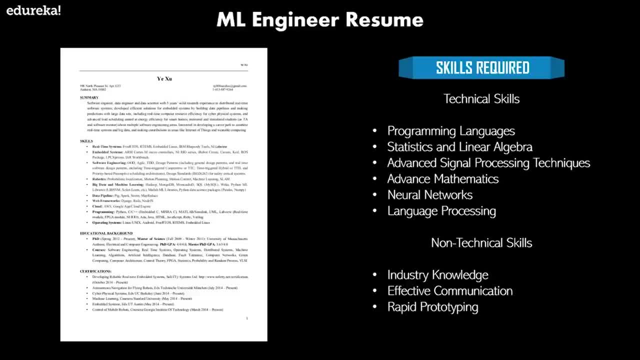 mandatory for finding the one that works in machine learning. this applies to everything from picking the right model to working on projects such as a, be testing and much more. now you need to do a group of techniques used to quickly fabricate a scale model of a physical part or assembly using 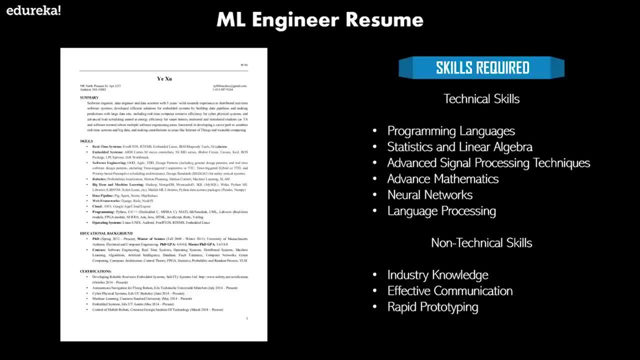 artificial computer aided design, which is the CAD data. now coming to the final skills which will be required for any machine learning engineer is to keep updated. now you must stay up to date with any upcoming changes. every month, new neural network models come out that outperform the 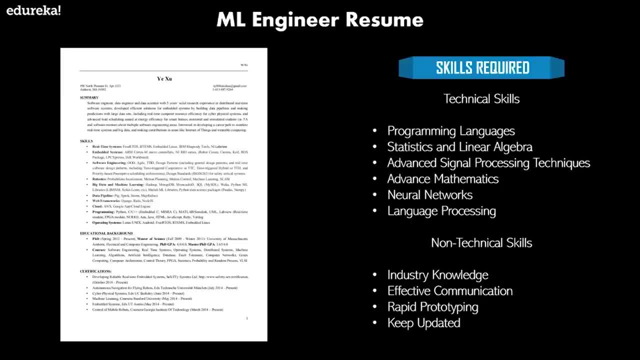 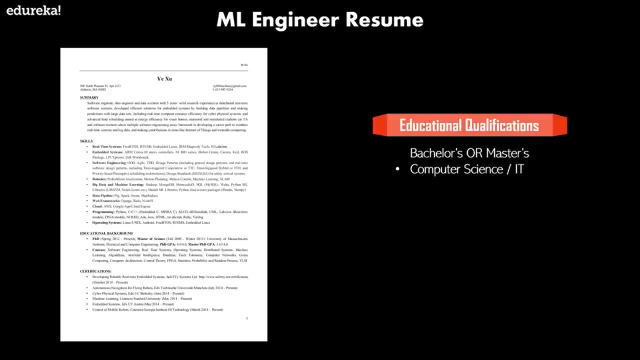 previous architecture. it also means being aware of the news regarding the development of the tools, theory and algorithms through research papers, blogs, conference videos and much more. now, another part of any machine learning engineer's is the educational qualification, so a bachelor's or a master's degree in computer science or IT. 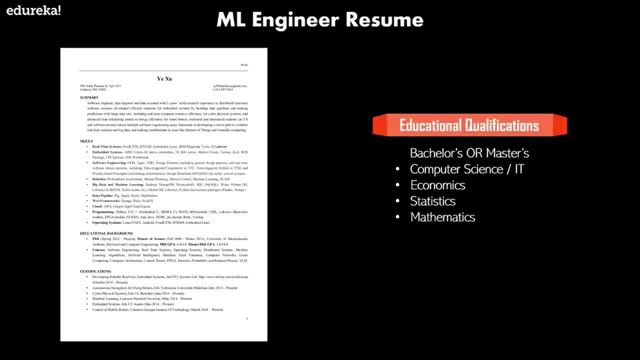 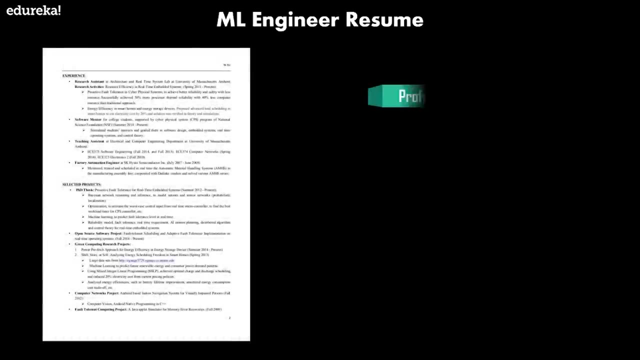 economics, statistics or even mathematics can help you land a job in machine learning. plus, if you are an experienced machine learning engineer, so probably some standard company certifications will help you a lot by landing a good job in machine learning. and finally, coming to the professional experience, you need to have experience in computer science, statistics, data asses, if you 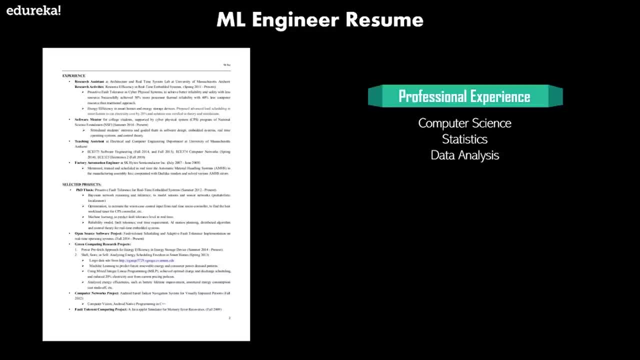 are from any other profession to a machine learning engineer, or if you have a previous experience in machine learning, that is very well. now, finally, if we talk about the projects, so you need to have not just any project that you have worked on. you need to have working on machine learning related. 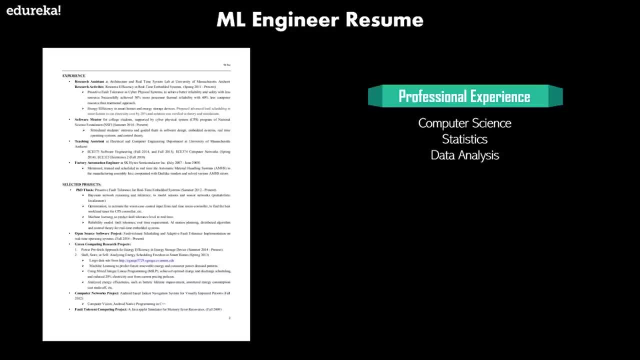 statistics, data asses. if you are switching from any other profession to a machine learning engineer, or if you have a previous experience in machine learning, that is very well now, finally, if we talk about the project, so you need to have not just any project that you have worked on. you need to have working on machine. 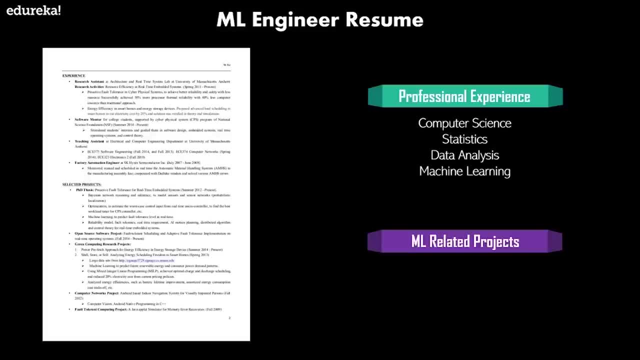 learning related projects that involve a certain level of AI and working on neural networks to a certain degree, to land a good job as a machine learning engineer. now, if we have a look at the company's hiring machine learning engineers, so every other company is looking for a machine. 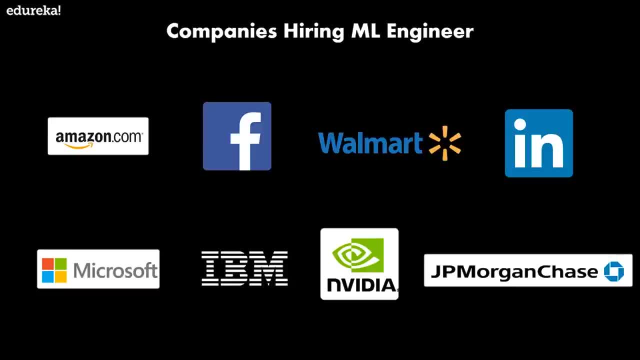 learning engineers who can modify the existing model to something that did not need much more of maintenance and can sustain. so, basically, working on artificial intelligence and new algorithms that can work on their own is what every company desires. so Amazon, Facebook. we have tech giants like Microsoft, IBM, again in. 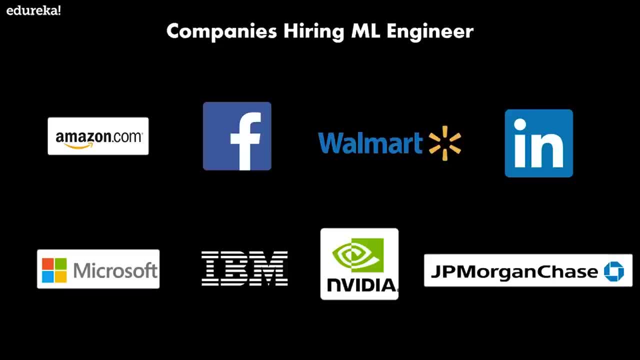 the gaming industry we have, or the GPU industry, graphics industry, we have Nvidia. in banking industry, we have JPMorgan Chase, again we have LinkedIn, and also we have Walmart. so all of these companies require machine learning engineer at some part of the times. so be sure that if you're looking for a machine learning engineer, post every other companies, be it a big. 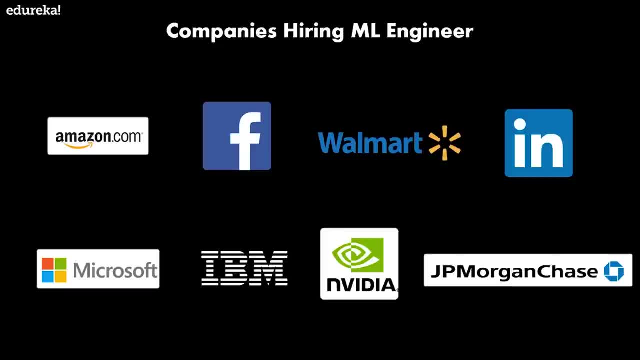 shot company, or even the new startups, are looking for machine learning engineers. so be assured you will get a job. now, with this, we come to an end of this video, so I hope you've got a good understanding of who exactly a machine learning engineer is the way. just job trends, the salary trends, what? 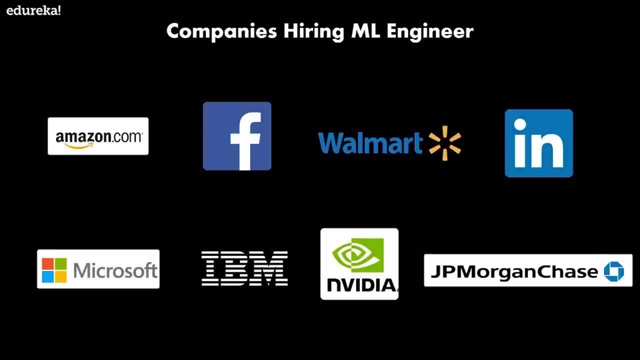 are the skills required to become a machine learning engineer and once you become a machine learning engineer, what are the roles and responsibilities or the job description, what appears be on the resume or the job description, what appears to be on the job application of any machine learning engineers? and also, i hope you got to know how to prepare your resume or how to 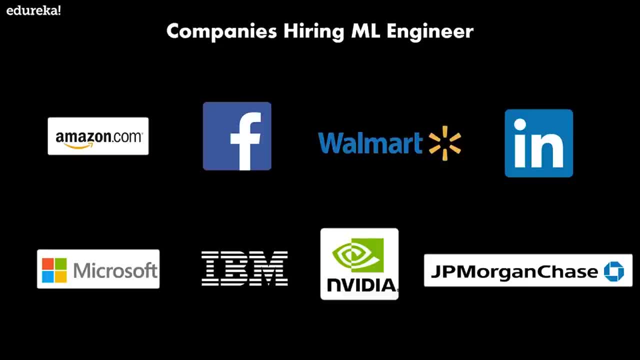 prepare it in a correct format and what all to keep there in the resume? the career objectives, the skills- technical and non-technical- previous experience, education, qualification and certain projects which are related to it. so that's it, guys. edureka, as you know, provides a machine learning. 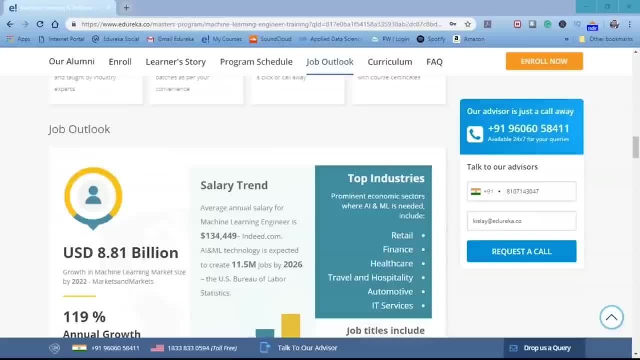 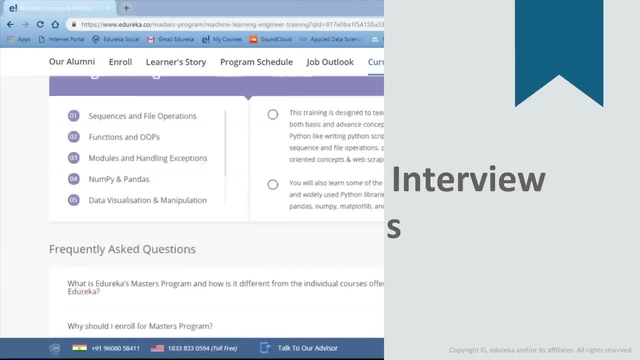 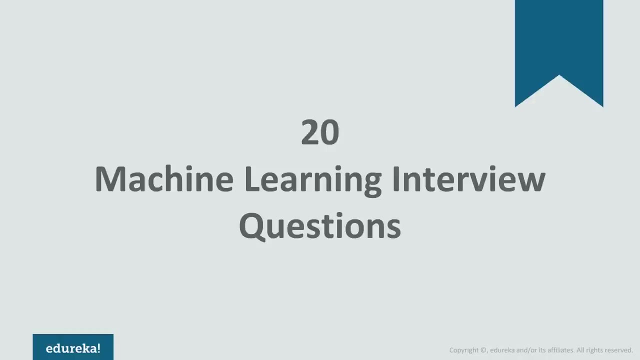 engineer master's program now that is aligned in such a way that will get you acquainted in all the skills that are required to become a machine learning engineer, and that, too, in the correct format as part of the machine learning interview series. i wanted to let you know that. 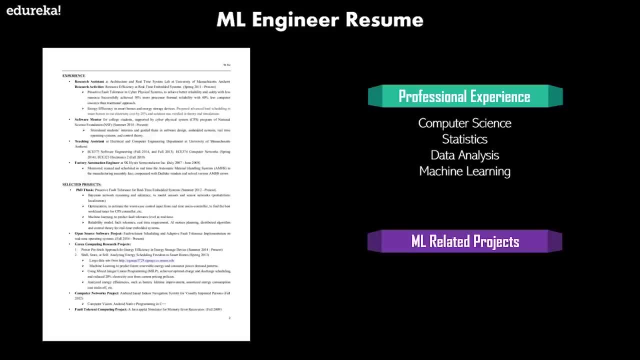 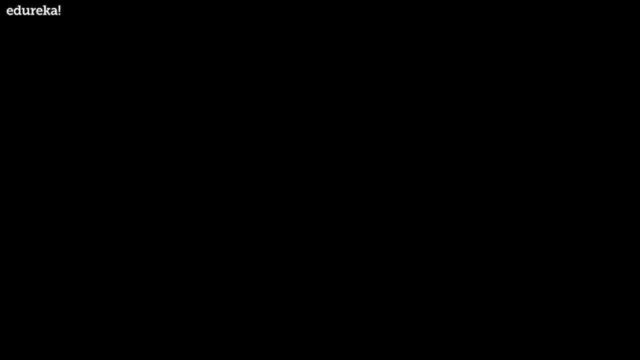 projects that involve a certain level of AI and working on neural networks to a certain degree, to land a good job as a machine learning engineer. now, if you have a look at the company's hiring machine learning engineers, so every other company is looking for a machine learning engineers who. 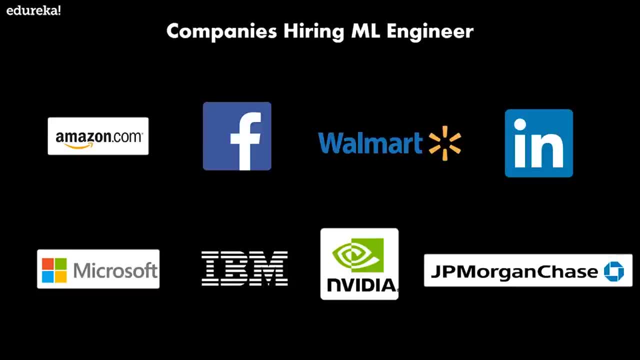 can modify the existing model to something that need not need much more of maintenance and can sustain. so, basically, working on artificial intelligence and new algorithms that can work on their own is what every company desires. so Amazon, Facebook- we have tech giants like Microsoft, IBM again. in the gaming industry, we have, or the GPU industry, graphics industry: we have Nvidia. 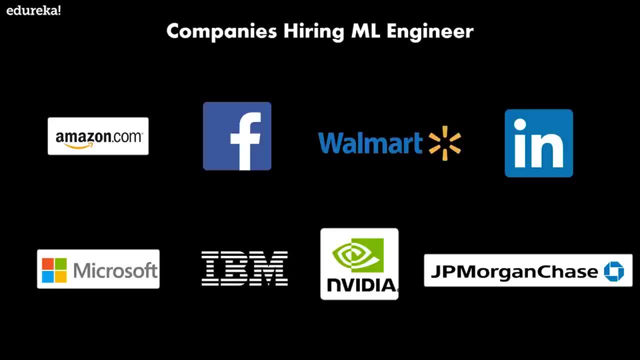 in banking industry. we have JPMorgan Chase, again we have LinkedIn and also we have Walmart. so all of these companies require machine learning engineer at some part of the times. so be assured that if you are looking for a machine learning engineer, post every other companies, be it a big. 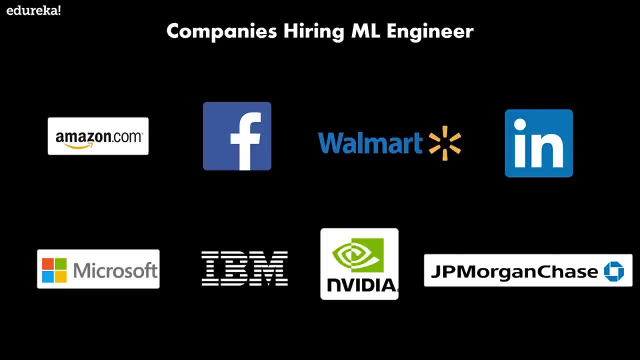 shot company, or even the new startups, are looking for machine learning engineers. so be assured you will get a job. now with this, we come to an end of this video, so I hope you've got a good understanding of who exactly a machine learning engineer is the way. just job. 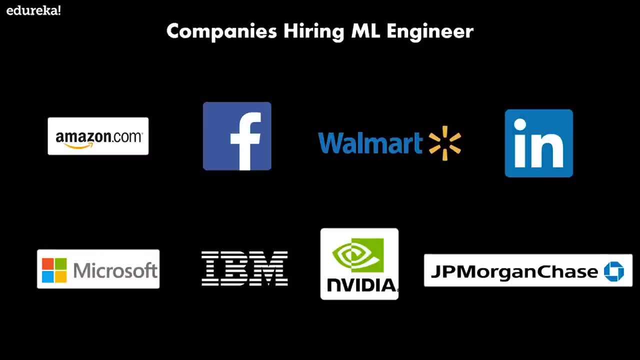 trends, the salary trends, what are the skills required to become machine learning engineer and once you become a machine learning engineer, what are the roles and responsibilities or the job description, what appears to be on the resume or the job description, what appears to be on the job application of any machine learning engineers? and also, I hope you got to know how to prepare. 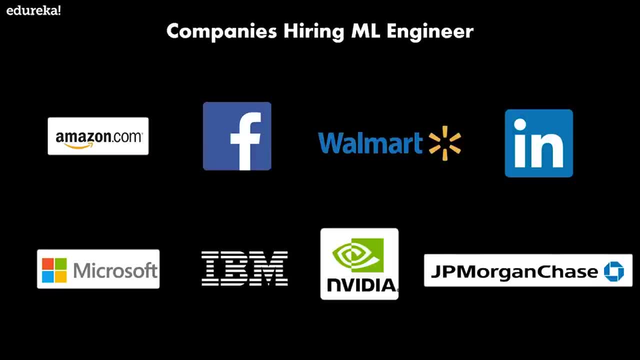 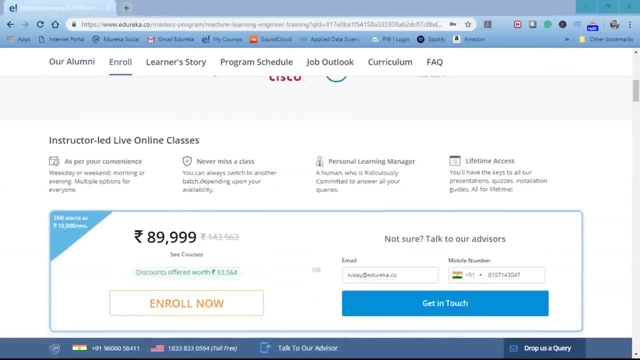 your resume, or how to prepare it in a correct format, and what all to keep there in the resume: the career objectives, the skills, the technical and non-technical previous experience, education, qualification and certain projects which are related to it. so that's it, guys. Edureka, as you know, provides a machine learning engineer master's program. now that is. 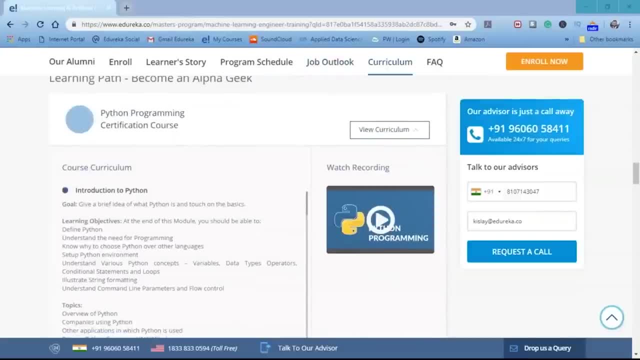 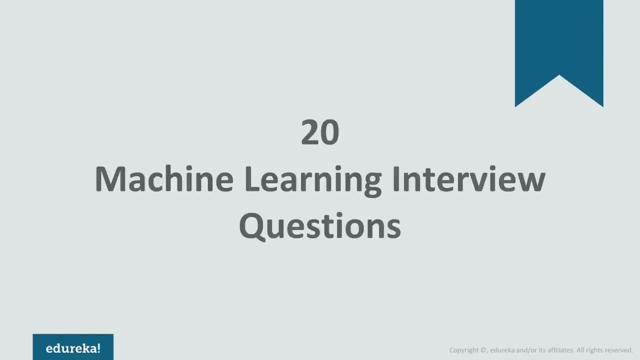 aligned in such a way that will get you acquainted in all the skills that are required to become a machine learning engineer, and that, too, in the correct format as part of the machine learning interview series. I wanted to let you know that would the market right now. the market right now. 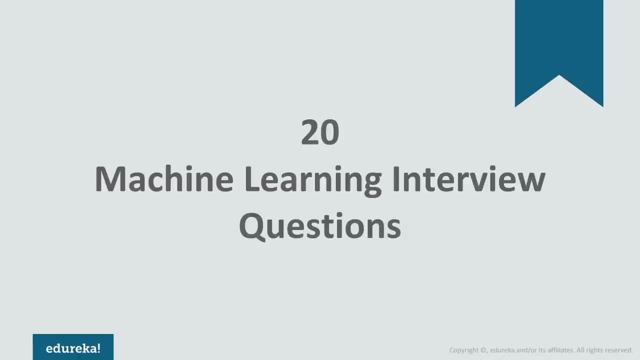 there is a lot of openings in the machine learning field, so every company is trying to use machine learning to understand and get gems from their data. they have a data, but they don't know what to do with their data, and they want machine learning engineers to have them understand the data so that 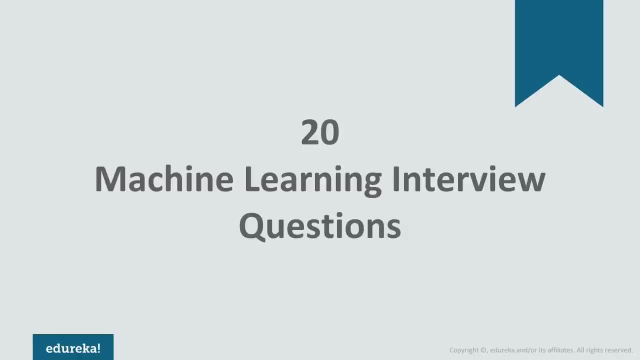 over the market. right now there is a lot of openings in the machine learning field, so every company is trying to use machine learning to understand and get gems from their data. they have a data, but they don't know what to do with their data and they want machine learning. 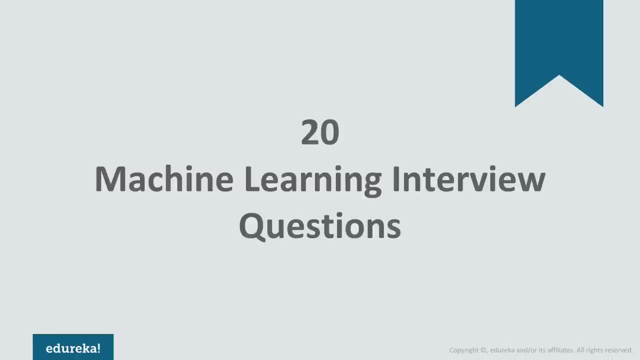 engineers, to have them understand the data so that their company revenues can be increased. so, on top of that, i wanted to also let you know that, over the openings, you will see that there are openings for data scientists, machine learning engineers, deep learning engineers, data analysts. many people are confused with the terms. as which one should we choose like? should we go with the? 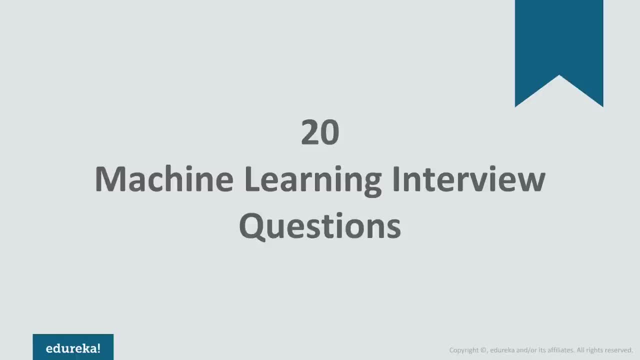 data scientists? should we go with the machine learning engineering? but these are all the terms that this company is used to attract some good talent. so this name they just use to attract the talent. but what you should focus is the job description. so what is the job description? 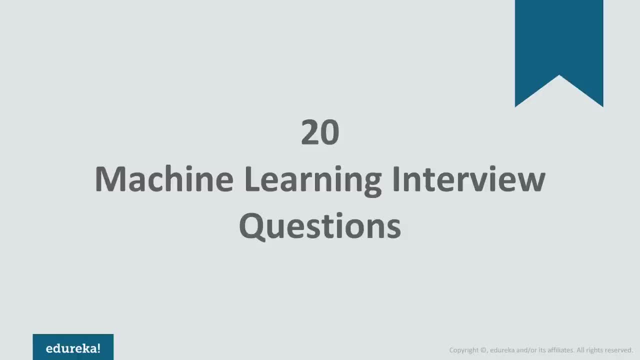 that they are providing and are you satisfied with that? so, whenever in the interview, try to ask the hr, try to ask the person who is taking the interviews what will be the rule and, based on that, take your decisions. names are okay, but what you're going to do. try to focus on that. so 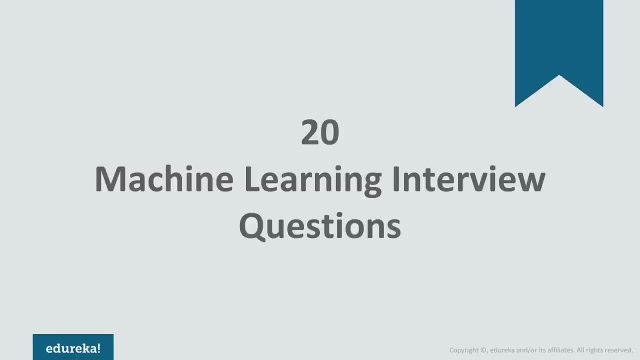 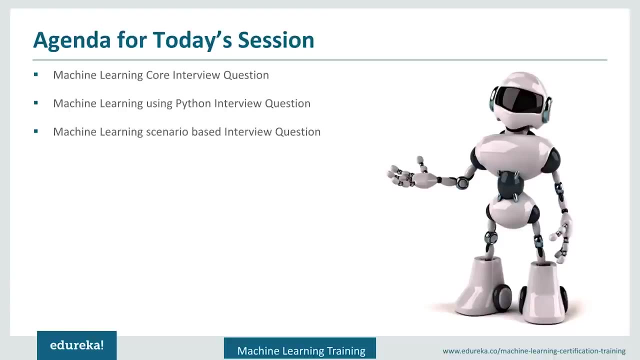 that is one thing that i wanted to let everyone know, because this is the thing that i see mostly in the internet that people are confused with. okay, so let's start with the interview questions. so first thing is, the session is divided into three components, so three broad. 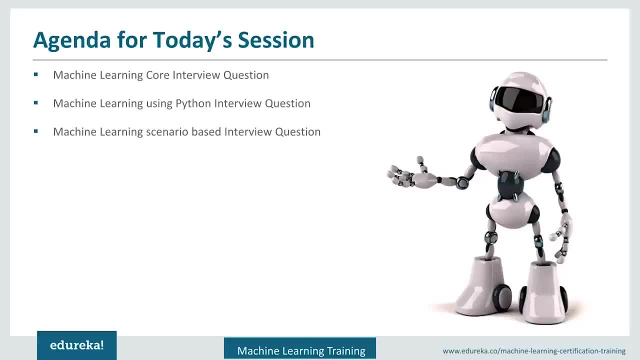 components. so first thing is machine learning: core interview questions. so within this core interview questions, we are more interested with the uh, the theoretical aspects of the machine learning, like how we're going to ask you the theoretical questions and you can explain those in an efficient manner. then second is the technical part, where we're going to 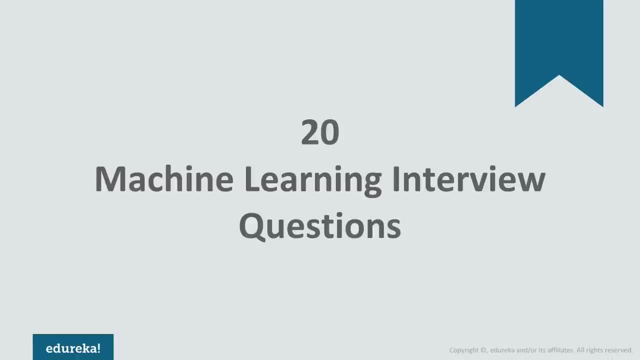 their company revenues can be increased. so, on top of that, I wanted to also let you know that over the openings, you will see that there are openings for data scientists, machine learning engineers, deep learning engineers, data analysts. many people are confused with the terms. as which one should we choose like? should we go with the? 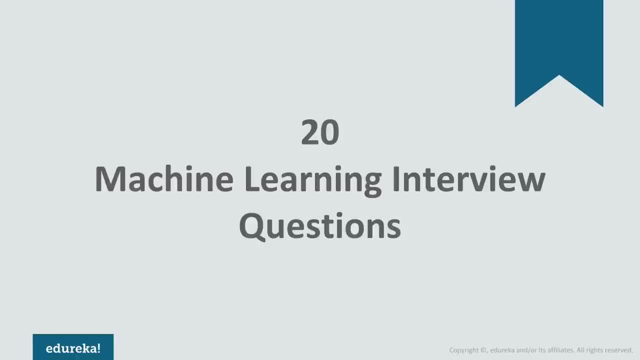 data scientists? should we go with the machine learning engineering? but these are all the terms that these companies use to attract some good talent. so this name they just use to attract the talent. but what you should focus is the job description. so what is the job description? that? 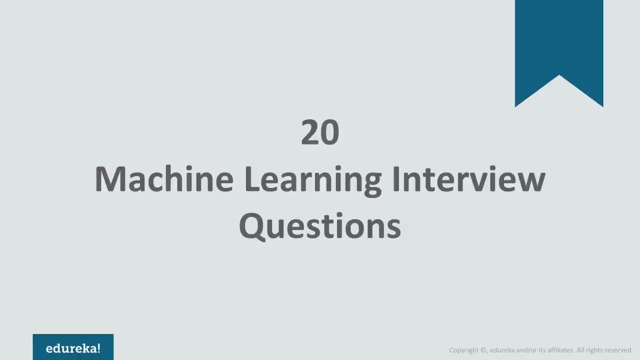 they are providing and are you satisfied with that? so, whenever in the interview, try to ask the HR, try to ask the person who's taking the interviews what will be the rule and, based on that, take your decisions. these names are okay, but what you're going to do, try to focus on that. so that is. 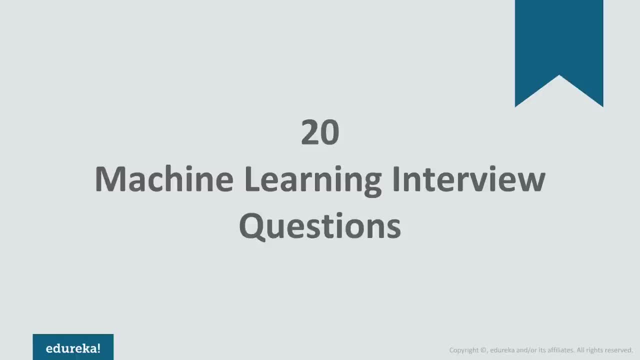 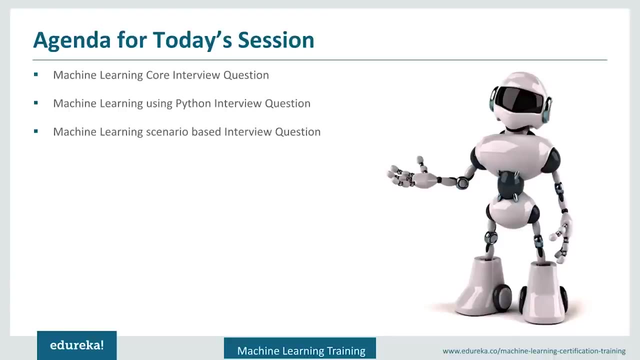 one thing that I wanted to let everyone know, because this is the thing that I see mostly in the internet that people are confused with. okay, so let's start with the interview questions. so first thing is, this session is divided into three components, three broad components. so first thing, 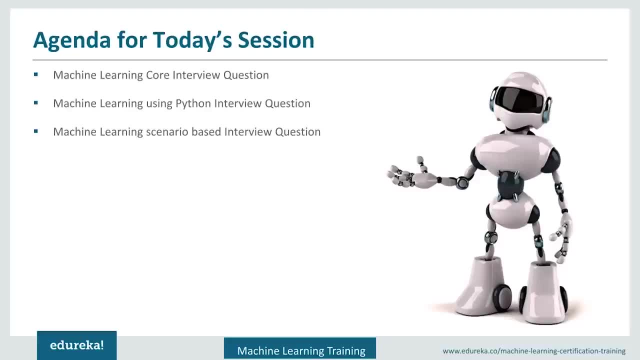 is machine learning core interview questions. so within this core interview questions we are more like how winter is going to ask you the theoretical questions and you can explain those in an efficient manner. then second is the technical part, where we going to see the interview questions related to the Python, so how we use the 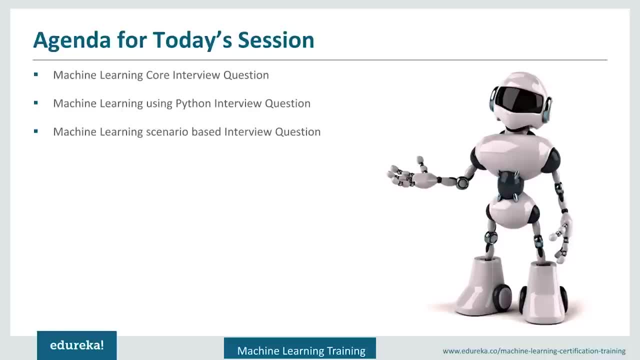 Python and the machine learning field. and last is the scenario based questions, so where the interviewer will be interested to see how you can solve the real-world problems using machine learning. so you will get some scenarios and based on the scenarios, you have to make your judgments and try to give the 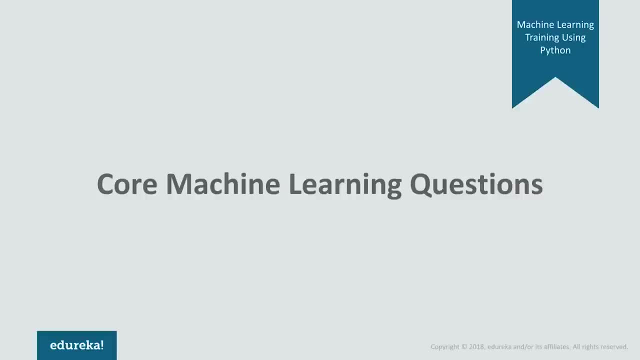 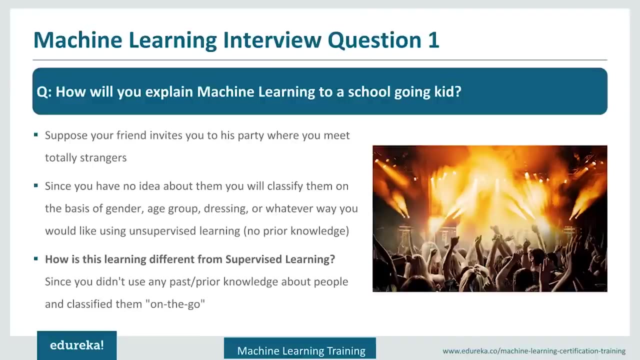 answers. so let's start with the core interview questions. first thing: how will you explain machine learning to a school going kid? so in this case the interviewer is interested to see how you can explain the concepts in machine learning in a very simple manner so that even a school going kid can understand. you can give an. 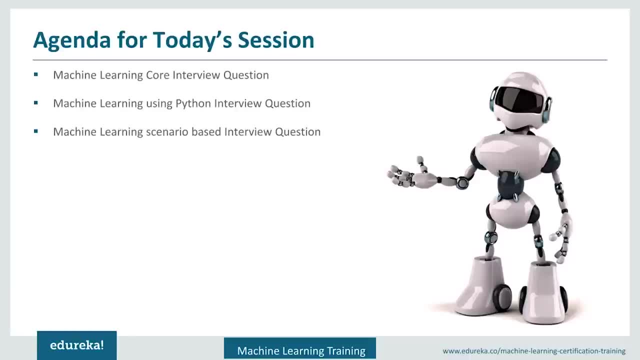 see the interview. questions related to the python, so how we use the python and the machine learning field. and last is the scenario based questions, so where the interviewer will be interested to see how you can solve the real world problems using machine learning. so you will get some. 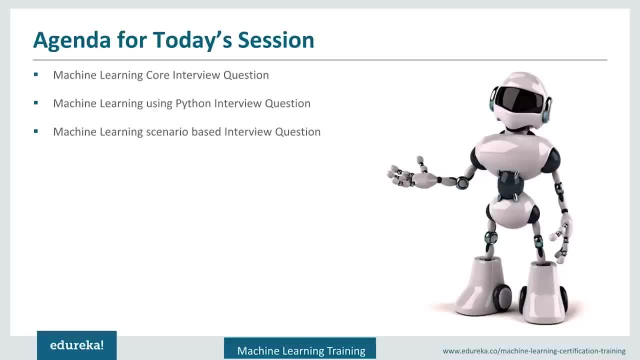 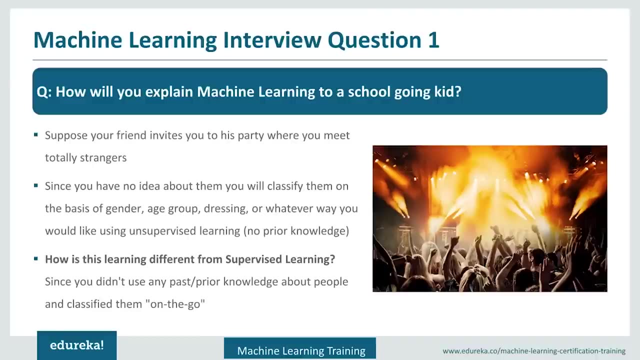 scenarios and based on the scenarios you have to make your judgments and try to give the answers. so let's start with the core interview questions. first thing: how will you explain machine learning to a school going kid? so in this case, the interviewer is interested to see how you can explain the concepts in 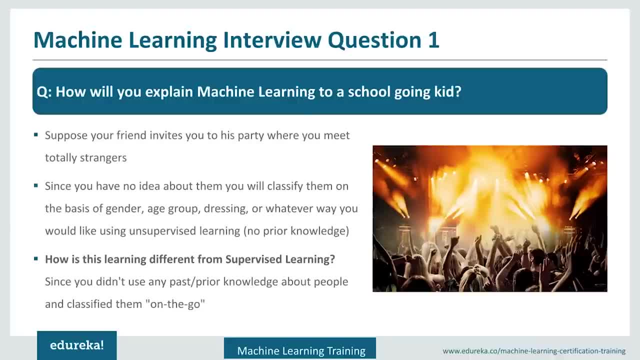 machine learning in a very simple manner so that even a school going kid can understand. you can give an example to a kid saying that, okay, your friend has invited you to a party and you meet completely strangers there. so you have not seen them previously, they are just completely. 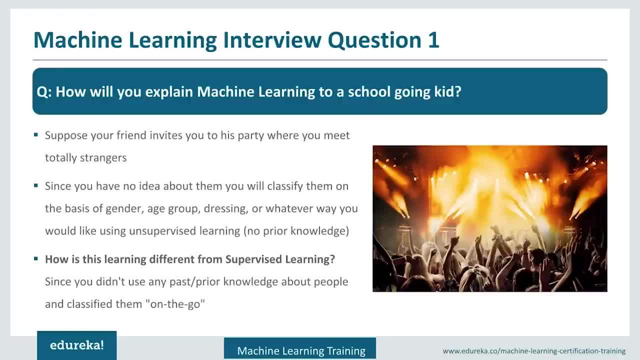 strangers to, and you're going to meet them, since you have no idea about them previously. so you will have to explain to them what you're going to do and how you're going to deal with them, based on the available things that you can visualize. that is like: what is the gender, what is the age group? 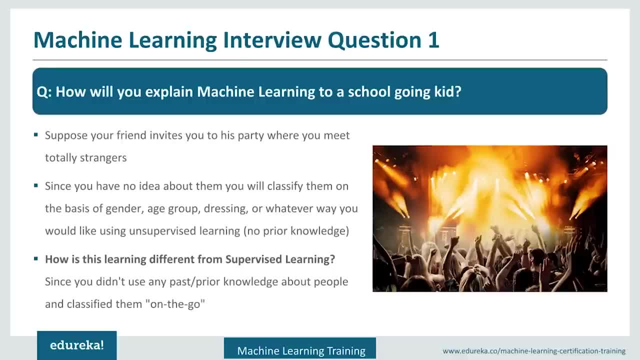 so how are they dressed, how do they behave with you like? what is their attitude? so he will try to classify them based on those features. so this is an pure example of unsupervised learning. so in this case we don't have any prior knowledge. so in this case they are completely, totally strangers. 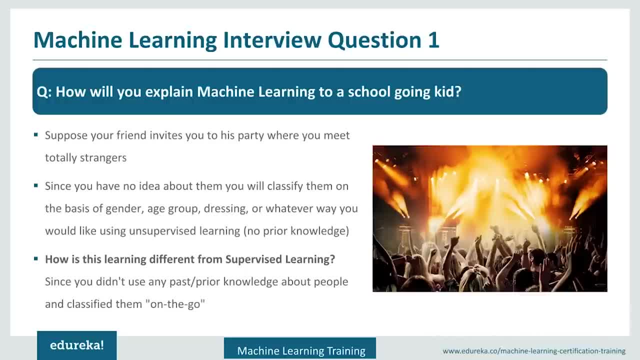 how is it different from the supervised learning? so in supervised learning the benefit will be: you will be able to classify them based on their age and based on that you will try to go so you can explain to the kid that, as you already got identified to those kids in future, you know. 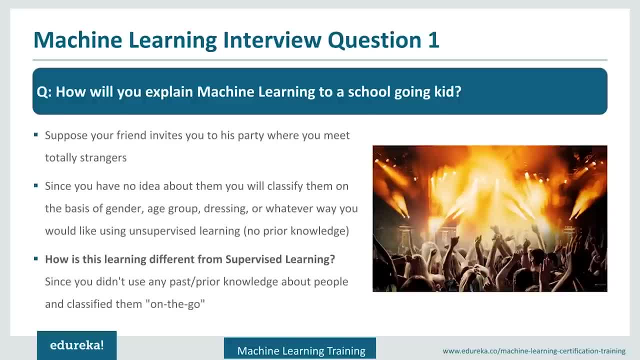 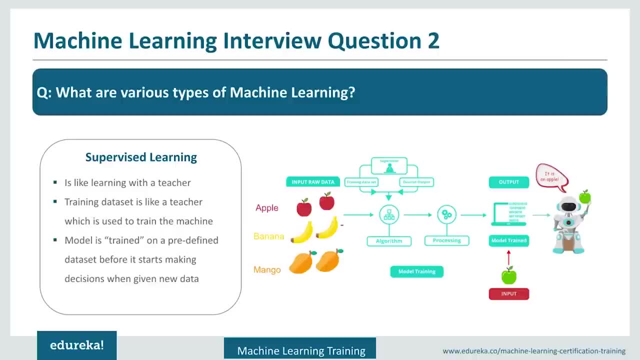 their names. so you will try to classify them whenever you see them. so that will be the example of supervised learning. so let's move on to the next thing: what are various types of machine learning? so first of all, you have to say that the machine learning is categorized into majorly three. 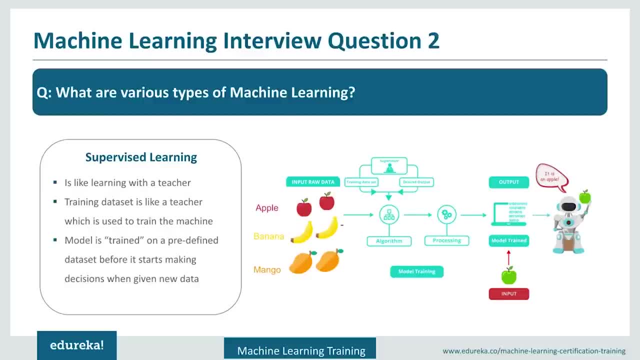 components: first is the supervised learning, second is the unsupervised learning and third is the forcement learning. so in the supervised learning it is like learning with a teacher, so training data set is like a teacher is giving you, like training the machine, so teacher is trying to train. 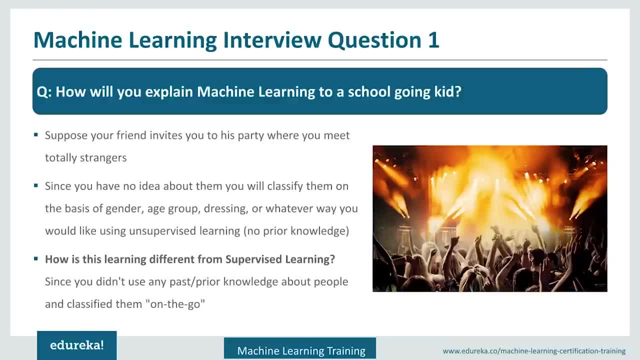 example, to a kid saying that, okay, your friend has invited you to a party and you meet completely strangers that so you have not seen them previously, they are just completely strangers to and you're going to meet them, since you have no idea about them previously. so you will try to classify them based on the 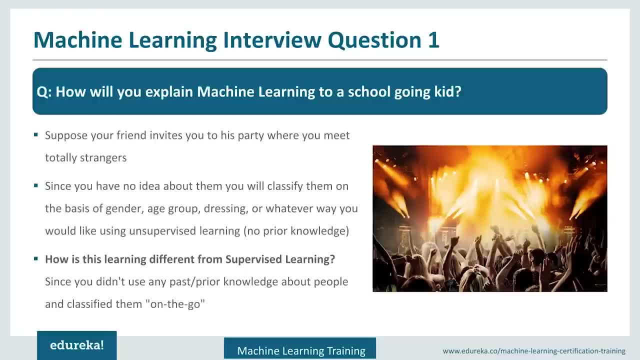 available things that you can visualize, that is like what is the gender, what is the age group? so how are they dressed, how do they behave with you? like, what is their attitude? so he will try to classify them based on those features. so this is an pure example of unsupervised learning. so in this 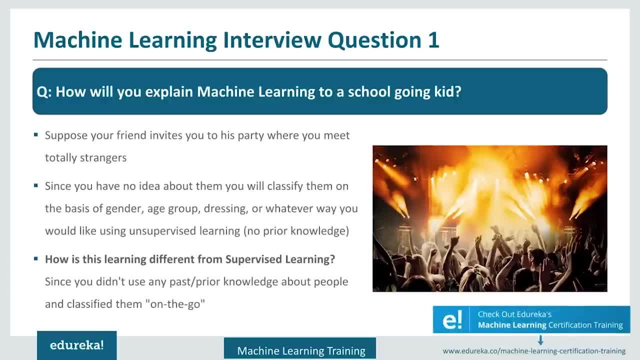 case we don't have any prior knowledge. so in this case they are completely, totally strangers. how is it different from the supervised learning? so in supervised learning the benefit will be you will have some prior knowledge and based on that you will try to go so you can explain to the kid that, as you 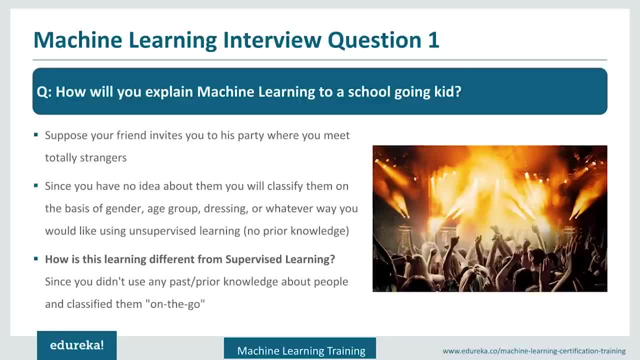 already got identified to those kids in future. you know their names, so you will try to classify them whenever you see them. so that will be the example of supervised learning. so let's move on to the next thing: what are various types of running? so first of all, you have to say that the machine learning is 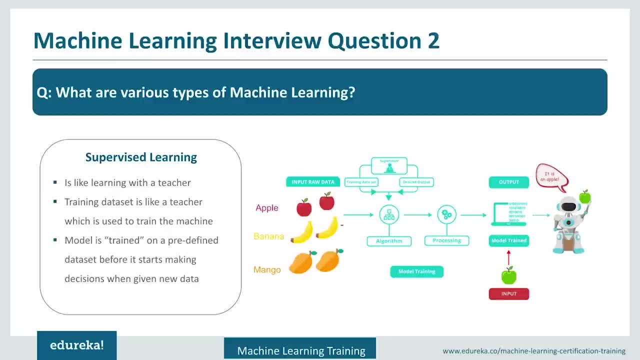 categorized into really three components: first is the supervised learning, second is the unsupervised learning and third is the reinforcement learning. so in the supervised learning it is like learning with a teacher, so training data set is like our teacher is giving you, like training the machine, so teacher is. 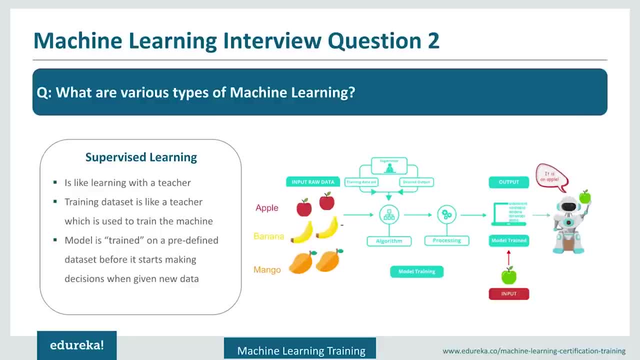 trying to train based on the whatever teacher knows. so, mother, like trained on the spreed, define data which you have and it start to make decisions based on the- again based on this rule that it has identified from the existing data, it will try to make some predictions and decisions on the new data. 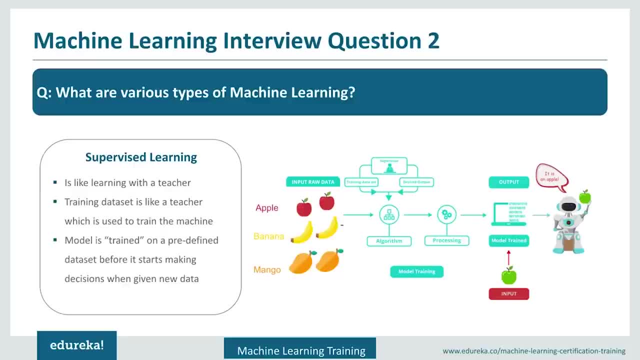 you can give some examples, as we have here in this case, when we have apples and bananas, we feed machine apples and bananas with the label saying that okay, this is the apple, this is how it looks, this is the one set of bananas and this is how they look. so when you feed it to the machine, 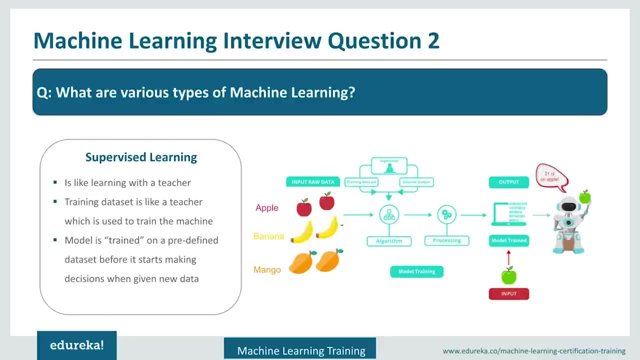 based on the whatever teacher knows so model is like trained on the speed defined data which you have and it start to make decisions based on the- again based on this rule that it has identified from the existing data. it will try to make some predictions and decisions on the new data you can. 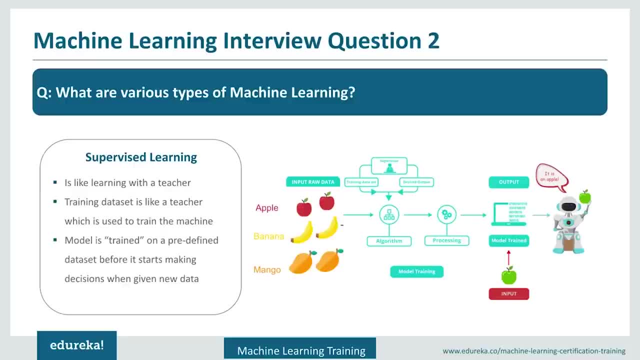 have here. in this case, when we have apples and bananas, we feed machine apples and bananas with the label saying that: okay, this is the apple, this is how it looks, this is the one set of bananas and this is how they look. so, when you feed it to the machine learning supervised algorithm, 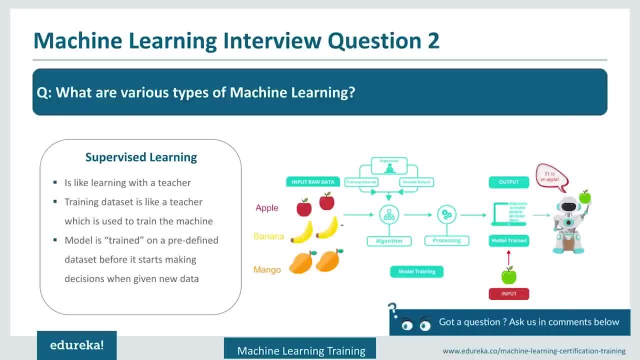 so what it does is it tries to identify the patterns which are there with each category. so it will say: it set the rule that, okay, apple looks like this, banana looks like this. so this is the model which is being provided, based on which our supervised learning learn set and we use this. 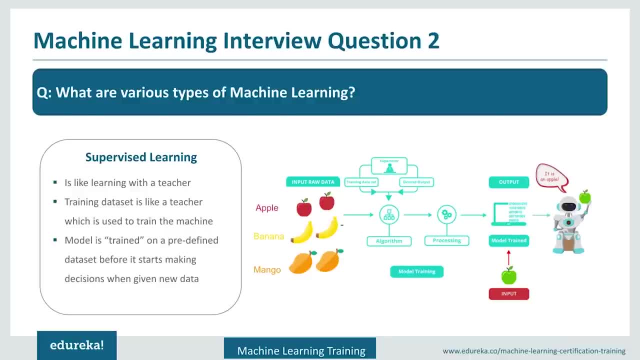 model on the new data set. so, for example, in this case we are using this green apple and, based on the structure which is already there, the green apple is still going to be predicted as an apple based on the shape it has. okay, so that is the example of supervised learning. let's move to the 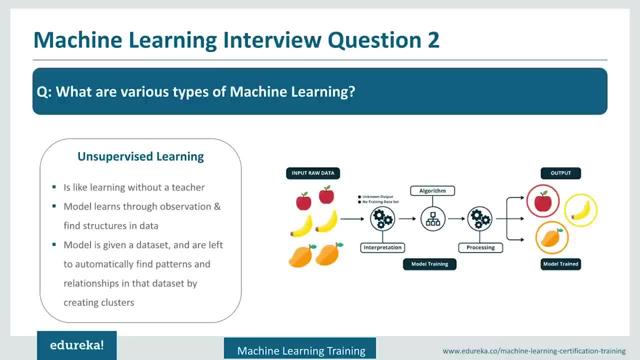 next thing, which is unsupervised learning. so in this case it is like learning without a teacher. so model learns through the observations which are there and it tries to identify some patterns and structure which will be hidden within the data. so in this case we are not labeling the data, so model is given a data and model is left on itself. 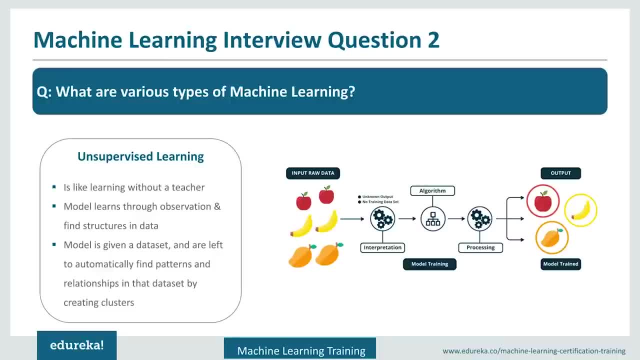 to learn the patterns and relationships out of the data by creating clusters. so clustering is one of the major techniques which are used in the unsupervised learning. there are many, but this is the most popularly used within the unsupervised. so, for example, when we feed the apples bananas. 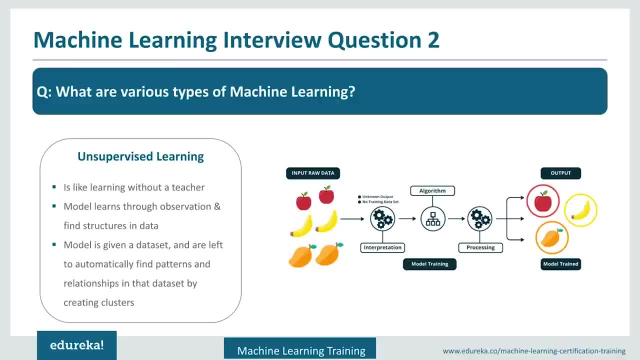 and the mangoes here again, but in this case we are not labeling them. we are not telling the machine that, okay, these are the apples, these are the bananas. we're just giving it the data, saying: okay, this is what it is. we don't know anything about it. so when we feed it to the 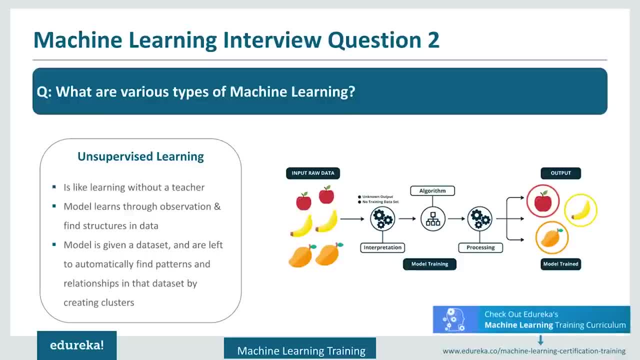 algorithm. algorithm tries to learn the patterns out of it and tries to classify them. it won't say: this is apple, this is banana, but it will say: okay, these are similar. so apples are similar and they'll try to cluster them together. bananas are similar. it will try to separate them in a different. 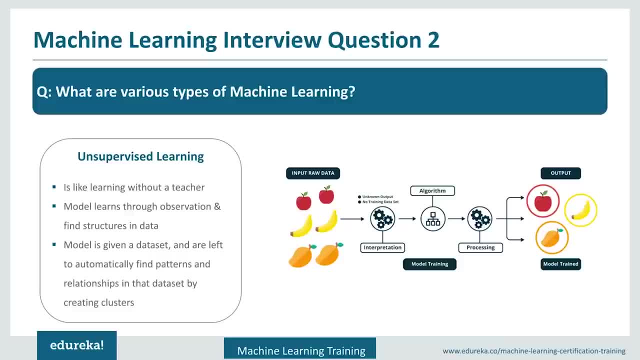 cluster and mangoes are similar, it will try to cluster them in a separate cluster. so it will try to understand the patterns which are there within the data and give you the clusters out of it. so that is the unsupervised learning. third part is reinforcement learning. so in this case, model. 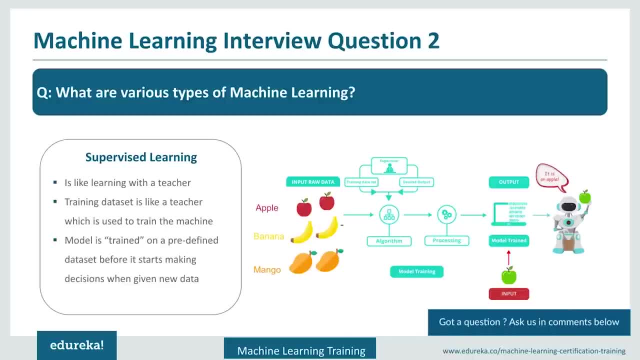 learning supervised algorithm. so what it does is it tries to identify the patterns which are there with each category. so it will say: it said the rule that, okay, apple looks like this, banana looks like this. so this is the training data that we have provided, based on which our supervised learning 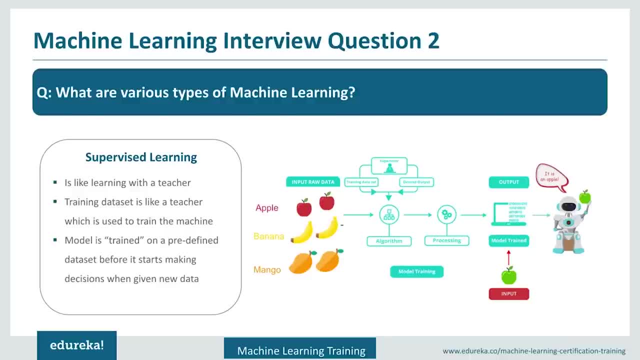 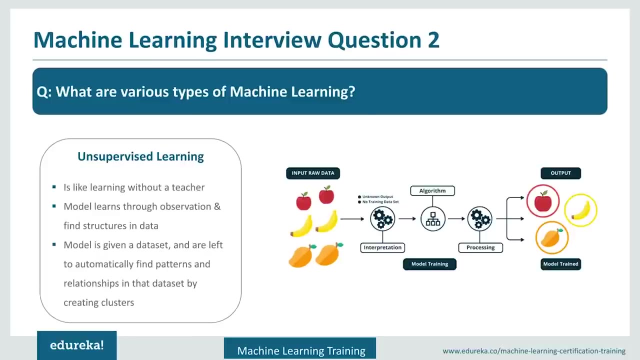 learn set and we use this model on the new data set. so, for example, in this case we are using this green apple and, based on the structure which is already there, the green apple is still going to be predicted as a apple based on the shape it has. okay, so that is the example of supervised learning. let's move to the 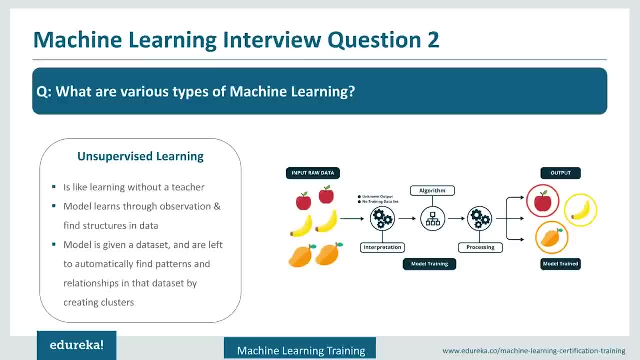 next thing, which is unsupervised learning. so in this case it is like learning without a teacher. so model learns through the observations which are there and it tries to identify some patterns and structure which will be hidden within the data. so in this case we are not labeling the data. so 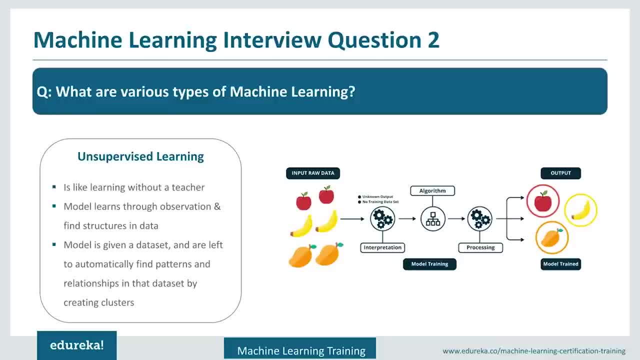 model is given a data and model is left on itself to learn the patterns and relationships out of the data by creating clusters. so clustering is one of the major techniques which are used in the unsupervised learning. there are many, but this is the most popularly used within the unsupervised. so 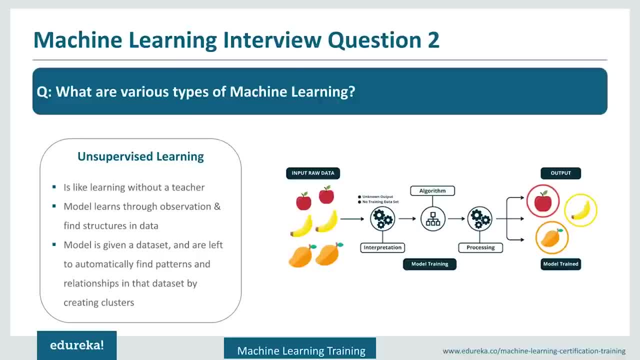 for example, when we feed the apples, bananas and the mangoes- here again, but in this case we are not labeling them, we are not telling the machine that, okay, these are the apples, these are the bananas. we just giving it the data, saying, okay, this is what it is, we don't know anything about it. so when 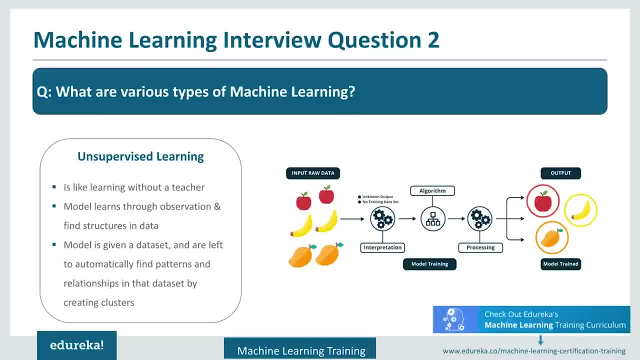 we feed it to the algorithm. algorithm tries to learn the patterns out of it and tries to classify them. it won't say this is apple, this is banana, but it will say, okay, these are similar. so apples are similar and they will try to cluster them together. bananas are similar. it will try to separate them in a different cluster. and mangoes? 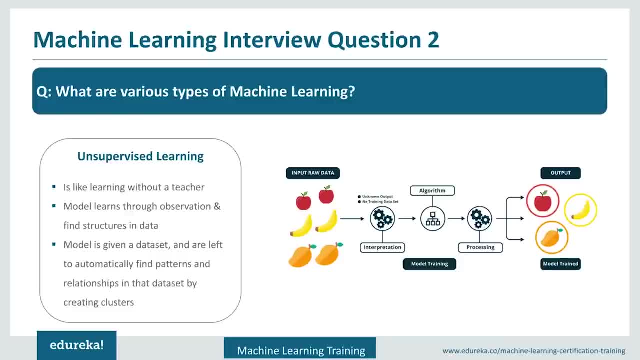 are similar, it will try to cluster them in a separate cluster. so it will try to understand the patterns which are there within the data and give you the clusters out of it. so that is the unsupervised learning. third part is reinforcement learning. so in this case model learns with hit. 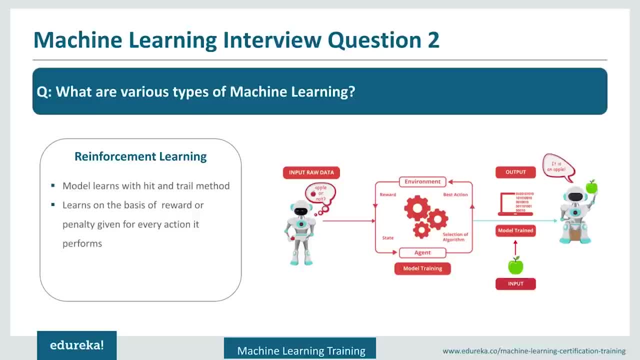 learns with hit and trial method. so assume that we are playing the mario game and in the mario game the player is called as the agent. in the reinforcement learning we have an environment which is a predefined action which agent can take. for example, in the game of mario it will be, he can move. 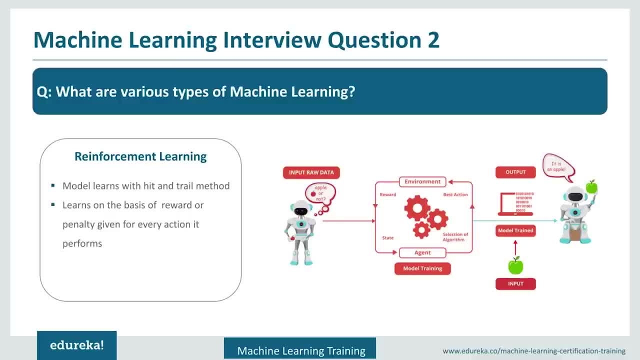 forward, he can jump, he can go into the tunnels, he can fire the bombs. so those are the steps and, based on these steps, your environment will try to reward you. either it will reward you or it will penalize you. based on that, your model will get created, which will say: okay, these are the best. 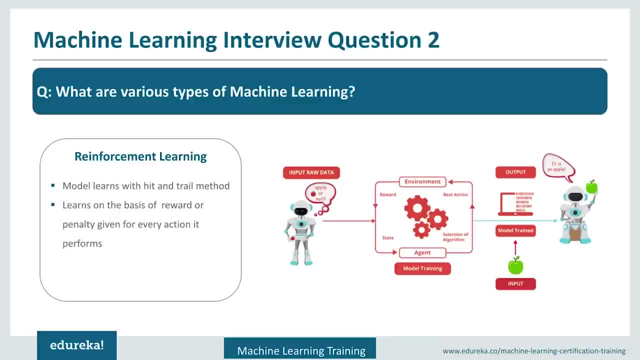 actions where when you do these actions, you will get your score more, which is like a reward, and don't you do this kind of action, your school will get penalized. so, based on this environment, your reinforcement learning will try to learn those things. so that is one example and you can also. 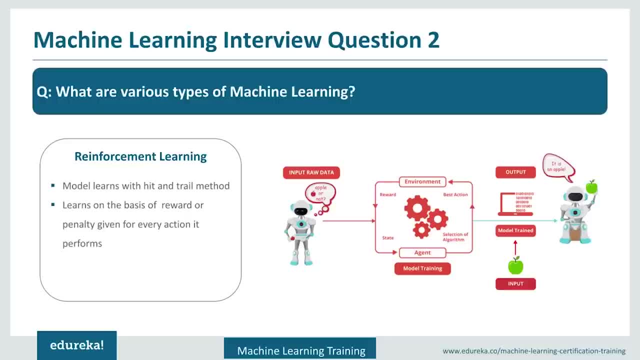 give some examples related to the alpha go, which is a go playing game which recently was developed by google based company. and you can also say that chess based games can be automated with the reinforcement learning. so there is one more category within machine learning, which is not much. 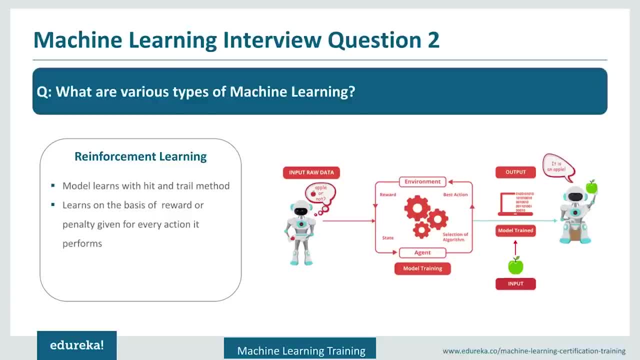 talked about, which is the semi-supervised learning and reinforcement learning. so this is the semi supervised algorithm, so which are basically combination of supervised plus unsupervised. so in this case what happens is you have a data set which is half of it is labeled and half of 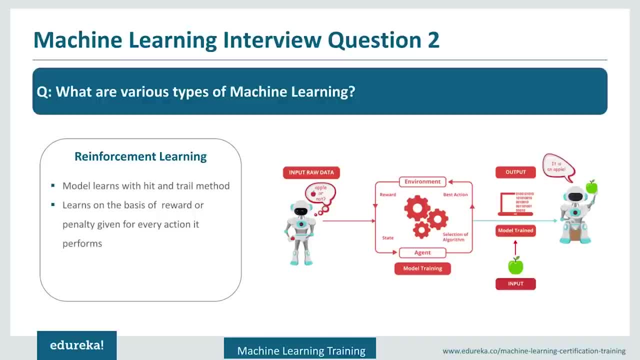 it is not labeled. so in this case, both supervised plus semi-supervised are used to create your models. so you can also give this, so that interview will be more confident on you, okay, so let's move on to the next thing. what's your favorite algorithm and can you explain it? 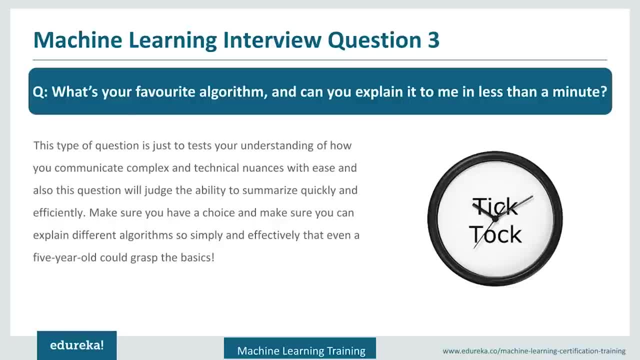 in a minute, in this case interview- is trying to understand as how you can explain some complicated techniques and technologies in a very simple and simplistic manner to some higher people or the clients or those kind of things. so make sure you have some choice and you can explain different algorithms in a simple manner. you keep for every example. try to keep some simple. 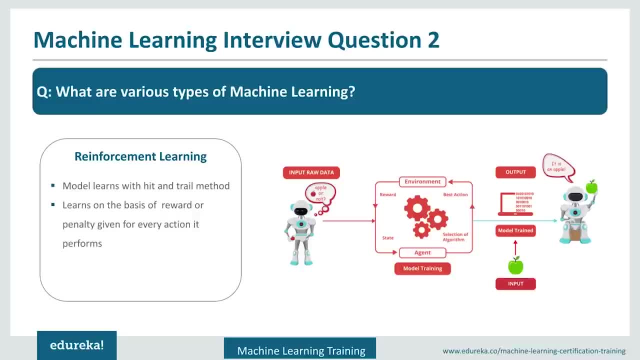 and trial method. so assume that we are playing the mario game and in the mario game the player is called as the agent. in the reinforcement learning we have an environment which is nothing but a game. there will be some predefined actions which agent can take, for example, in the game of 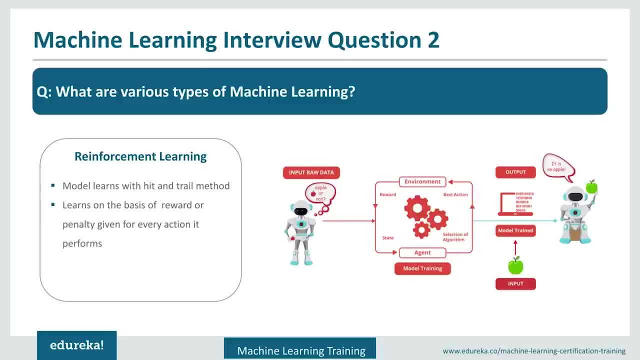 mario it will be. he can move forward, he can jump, he can go into the tunnels, he can fire the bomb. so those are the steps and, based on the steps, your environment will try to reward you. either it will reward you or it will penalize you. based on that, your model will get created, which will 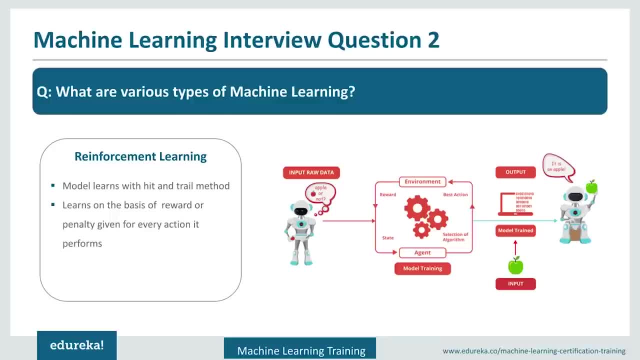 say: okay, these are the best actions, where when you do these actions, you will get your score more, which is like a reward, and when you don't, you do this kind of action, your school will get penalized. so, based on this environment, your reinforcement learning will try to learn those things so that 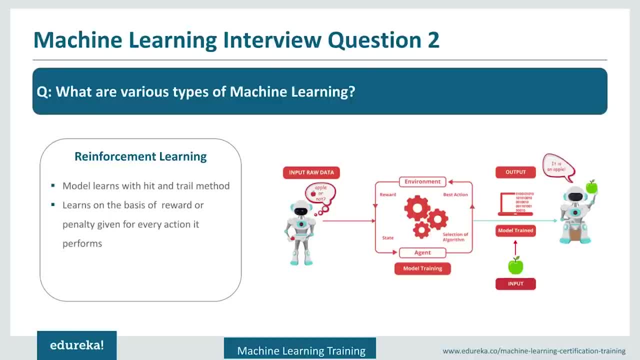 is one example and you can also give some examples, some examples related to the alpha go, which is a go playing game which recently was developed by google based company. and you can also say that chess based games can be automated with the reinforcement learning. so there is one more category within machine learning which is not 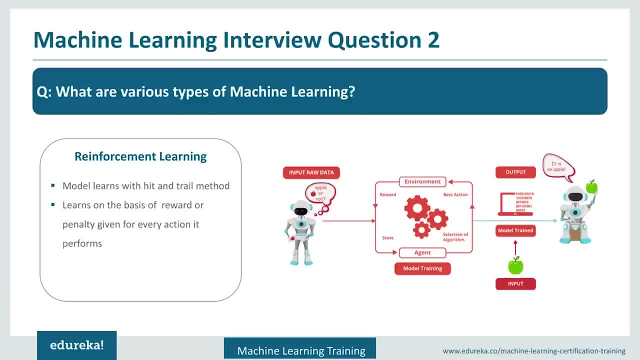 much talked about, which is the semi-supervised algorithm, so which are basically combination of supervised plus unsupervised. so in this case what happens is you have a data set which is half of it is labeled and half of it is not labeled, so in this case, both supervised plus semi-supervised. 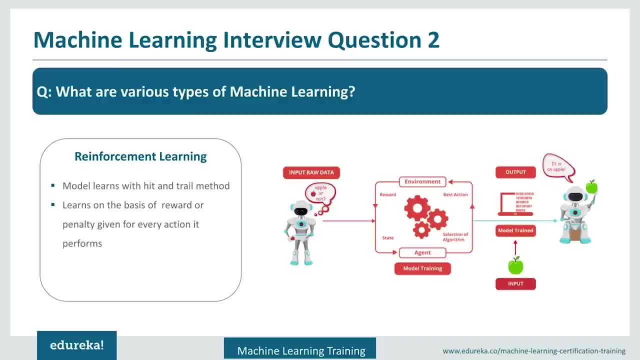 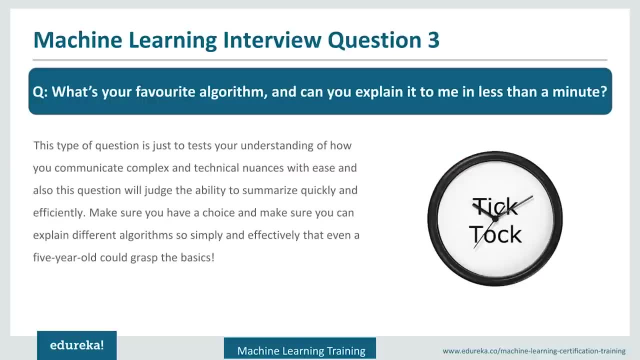 are used to create your models, so you can also give this, so that interview will be more confident on you, okay? so let's move on to the next thing: what's your favorite algorithm and can you explain it in a minute? in this case, interview is trying to understand as how you can explain some complicated 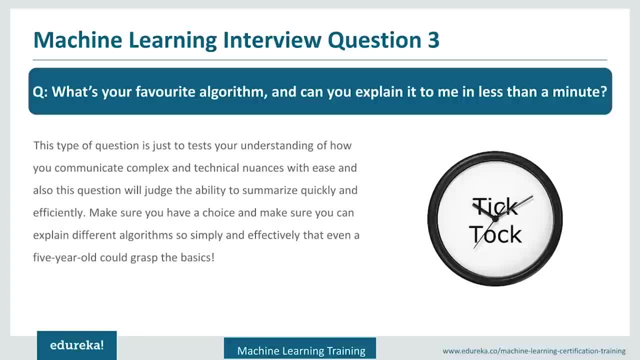 techniques and technologies in a very simple and simplistic manner to some higher up people or the clients or those kind of things. so make sure you have some choice and you can explain different algorithms in a simple manner. you keep for every example. try to keep some simple examples so that 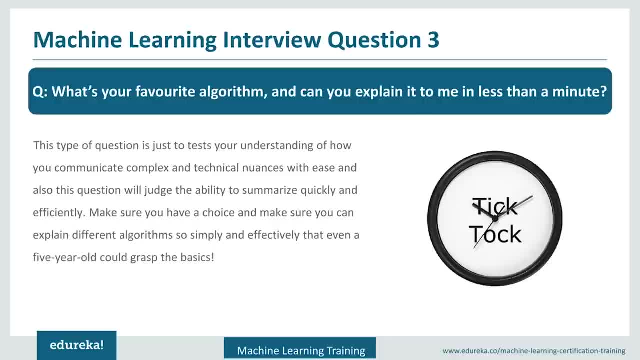 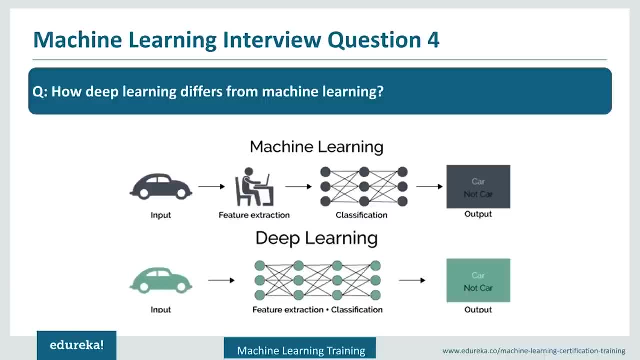 you can effectively and you can easily explain it so that even a small kid can understand as how you are explaining those things. so how deep learning is different from machine learning in this case. first thing is, you have to know that deep learning is not completely different from. 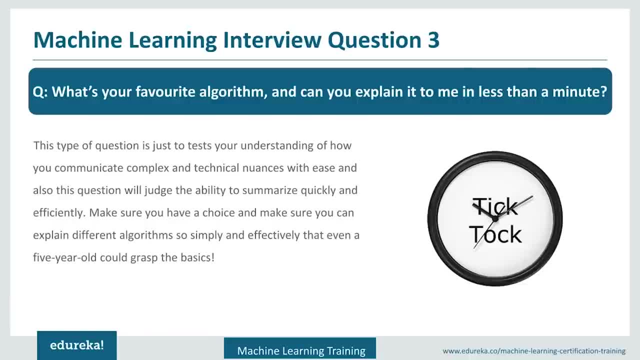 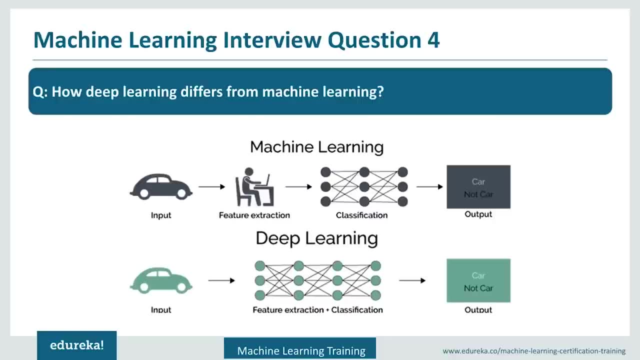 examples so that you can effectively and you can easily explain it, so that even a small kid can understand it as how you are explaining those things. so how deep learning is different from machine learning in this case? first thing is you have to know that deep learning is not completely different from machine learning. you have to say 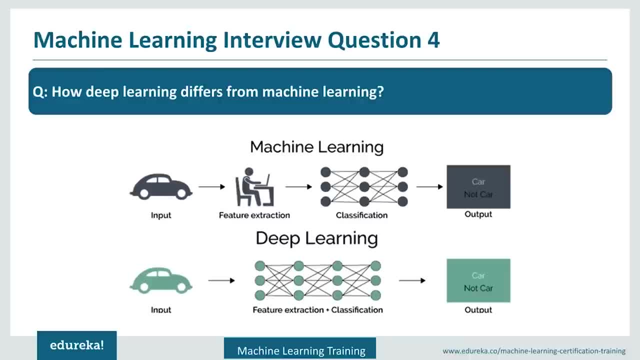 that okay. deep learning is a small part of machine learning and, in the core, machine learning based on the input. first you have to do the feature extractions. you have to classify the features which are the good, which are trying to explain your model better, based on some exploratory data analysis. 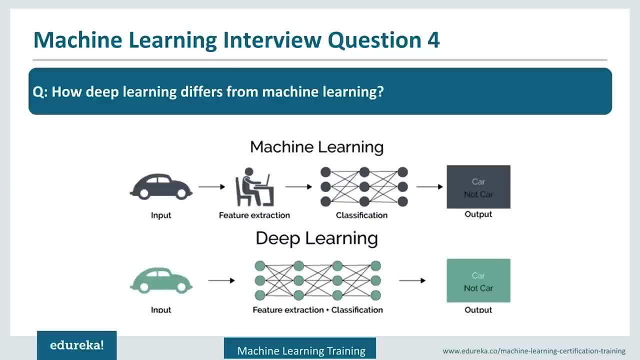 and based on that you will feed it to the algorithms and those algorithms will try to identify the patterns within those and give you the output. in deep learning it is bit simplified. what happens is based on the input. the model will try to extract the features on itself and will try to create a model. 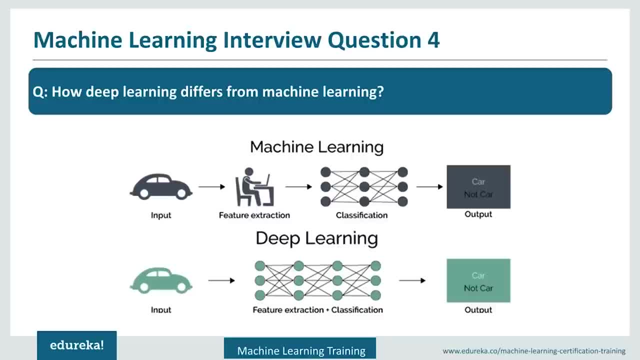 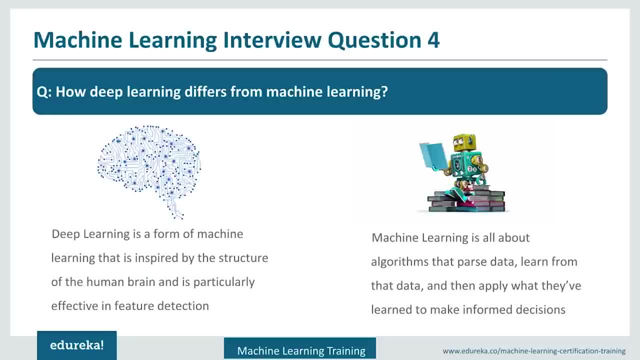 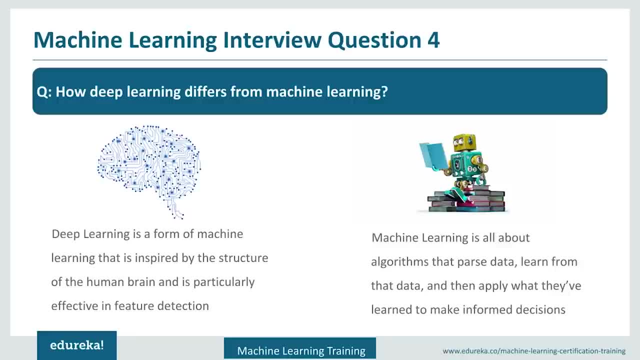 brain works and how the neurons within the brain really works in a very complicated and effective manner. so those are the things which have been taken and being implemented in the deep learning and machine learning is an. learning is about the algorithms that basically parses and learns the data and 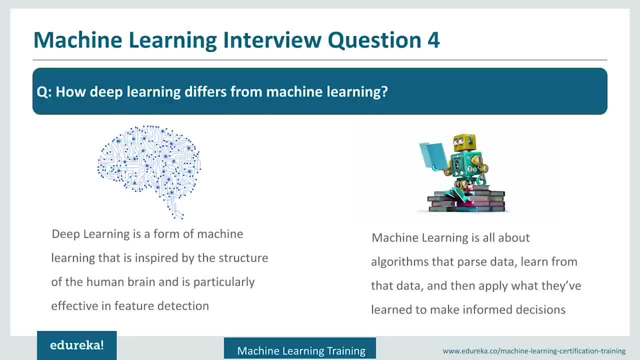 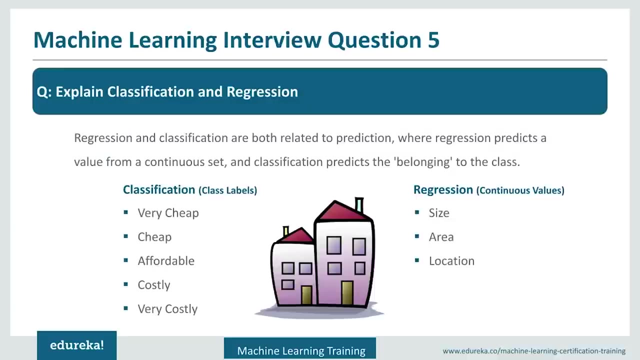 tries to identify the patterns within the data, apply whatever pattern learn from the data to the new data, whichever is coming. so that is the most of the thing which was related with the machine learning, but deep learning has come a bit more advanced to it. okay, so explain classification and regression. so 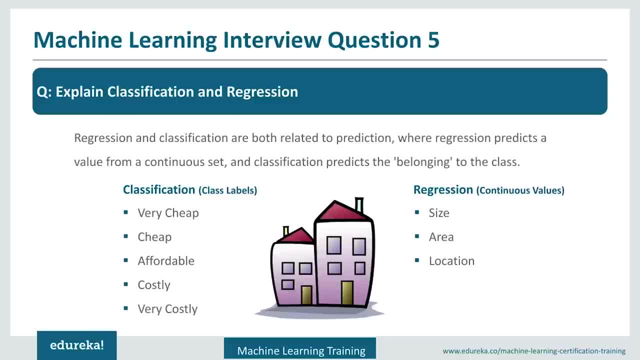 classification and regression is part of supervised learning. so you have to see this first, that this is part of the supervised learning. super was learning is broadly categorized into this two parts, and regression is mostly dealing with the continuous variable. so in continuous variable it's like you are. 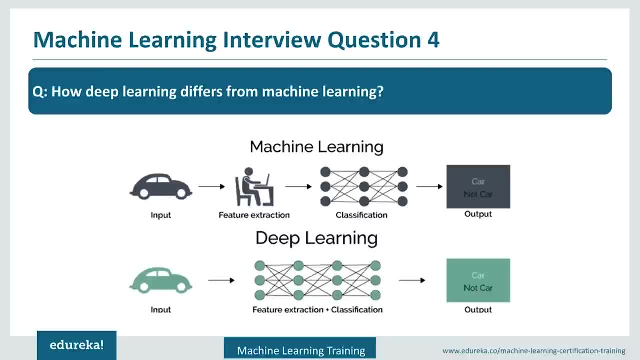 machine learning. you have to say that. okay, deep learning is a small part of machine learning and, in the core, machine learning based on the input. first you have to do the feature extractions. you have to classify the features which are the good, which are trying to explain your model better, based on some exploratory. 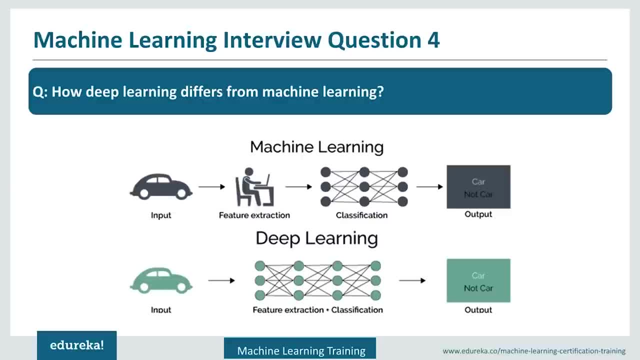 data analysis and based on that, you will feed it to the algorithms and those algorithms will try to identify the patterns within those and give you the output. in deep learning it is bit simplified. what happens is based on the input. the model will try to extract the features on itself and will try to create a model based on. 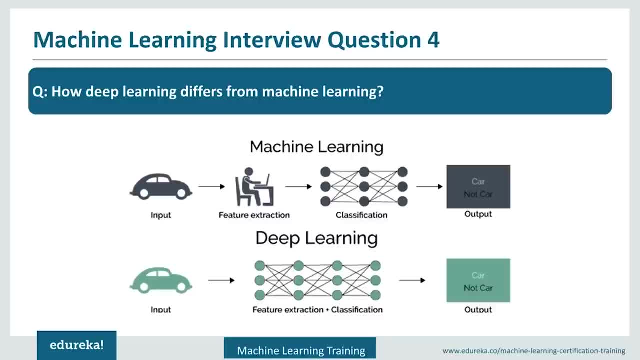 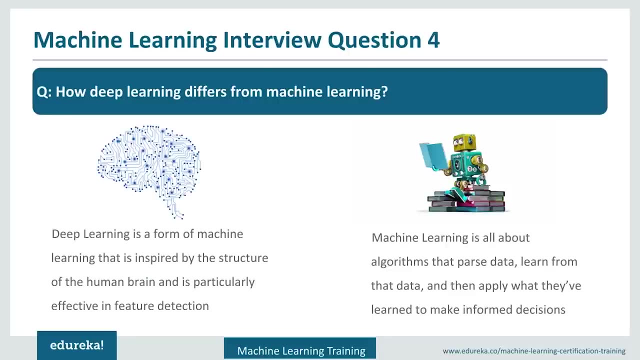 those. so it is trying to combine both the things of feature extraction and classification into a single thing and it will give you the output. so that's why it is recently being very popular. so that is one thing, and deep learning is basically. if you know, the deep learning is constructed most. 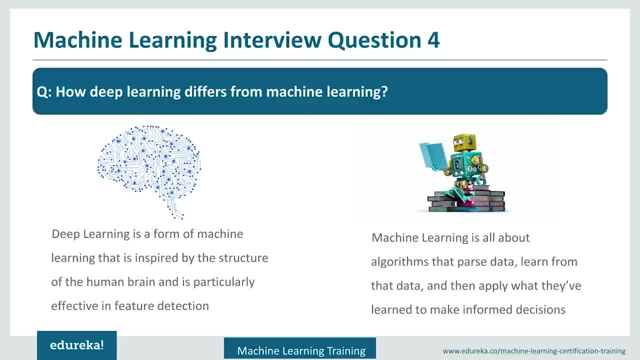 of the neural networks. so a neural networks are basically the neural networks that are used to run the data, and they basically borrowed from the idea of the human brain, so how the human brain works and how the neurons within the brain really works in a very complicated and effective manner. 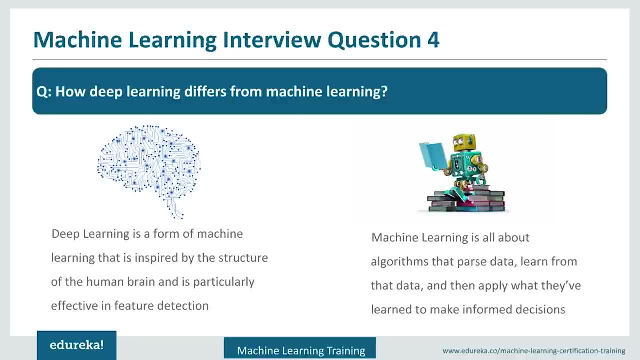 so those are the things which have been taken and being implemented in the deep learning, and machine learning is about the algorithms that basically parses and learns the data and tries to identify the patterns within the data, apply whatever pattern learned from the data to the new data. So that is the most of the thing which was related with the machine learning. but deep 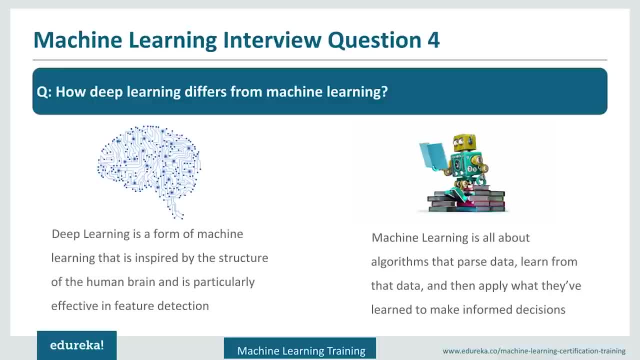 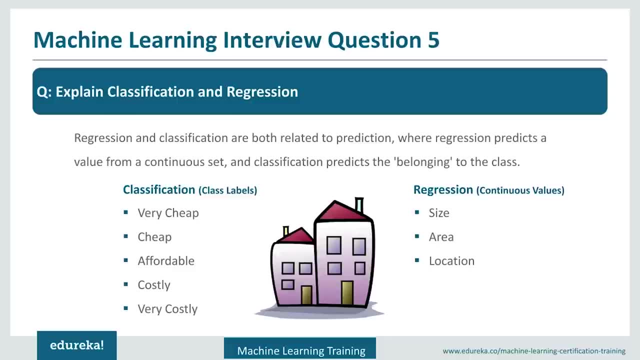 learning has come a bit more advanced to it. Okay, So explain classification and regression. So classification and regression is part of supervised learning. So you have to see this first, that this is part of the supervised learning. Supervised learning is broadly categorized into this two parts, and regression is mostly. 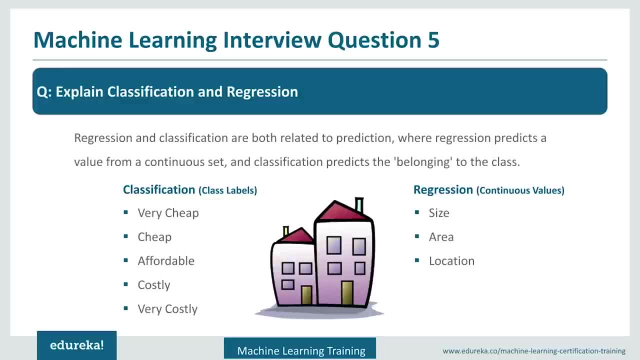 dealing with the continuous variable. So in continuous variable it's like you're trying to predict the sales, you're trying to predict the stock market values. So wherever there are continuous predictions, you're trying to do the regression of your data. So classification is like you're trying to predict the different classes which are there. 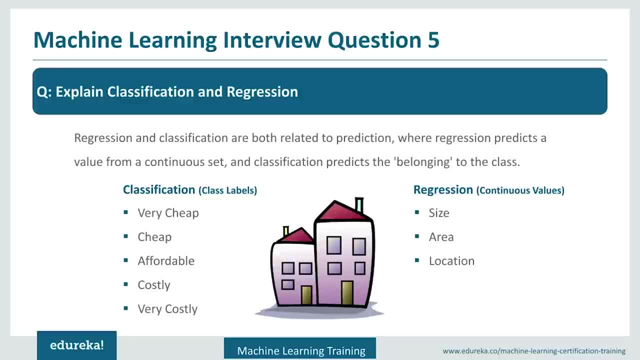 trying to predict the sales, you are trying to predict the stock market values. so wherever there are continuous predictions, you are trying to do the regression of your data. so classification is like: you are trying to predict the different classes which are there within the data. so, for example, if you are trying to predict the sales, you are trying to predict the. 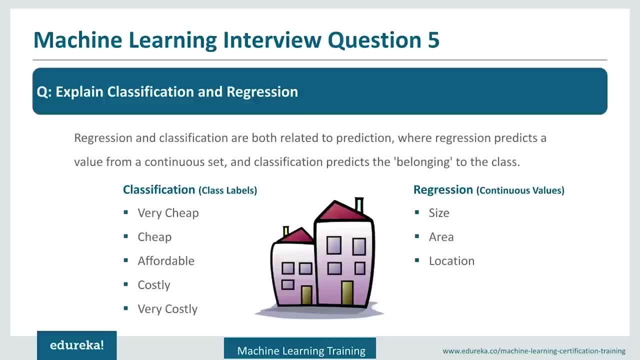 for example, the classes could be like: is the student going to pass or not, is my customer going to buy my product or not, and if my salary is within like high, medium, low? so those are the different classes, and when we're dealing with the classes, we say it is classification and we're dealing with the continuous values. 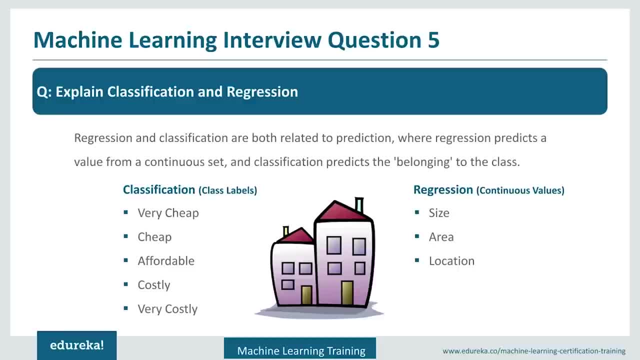 we say it is regression. so in this case, if you see, the regression is like size of your house, area and the location which are there, and the classification is like when you are trying to give it a classes: so very cheap, cheap, affordable, so you are creating a five classes here and that. 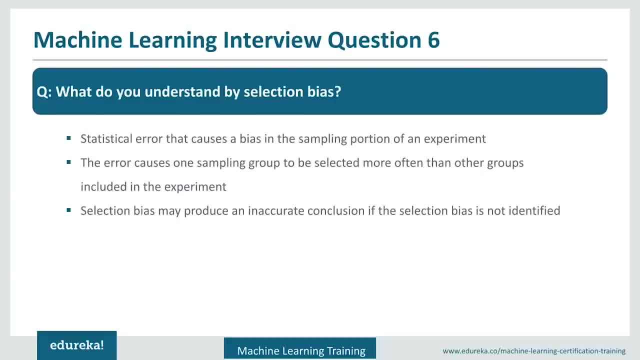 becomes a classification. what do you understand by selection bars in the statistical term? sampling is basically trying to sample some data from your population. so you are trying to take some portion of the data from the population and when you have some bias to some specific set of data, so let's. 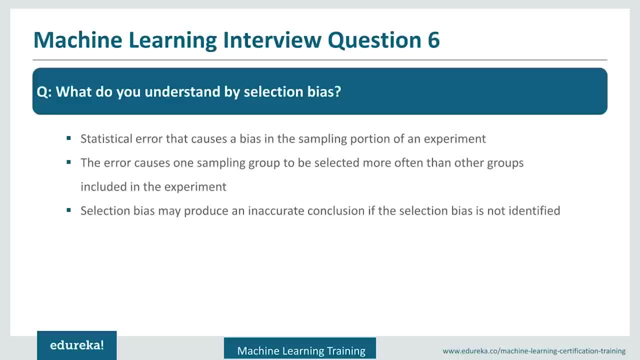 assume we want to take a population of offcolon, the data scientists within india. when you're talking about india, you have to take data from all parts of india. but let's assume you just take the sample from the gurgaon. so when you just take the sample from the gurgaon, you're getting a selection bias, you're getting bias to the gurgaon. 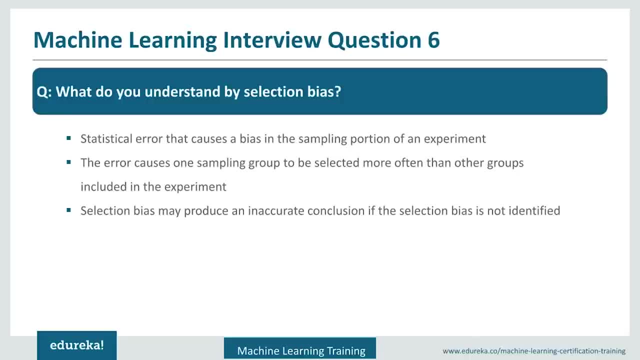 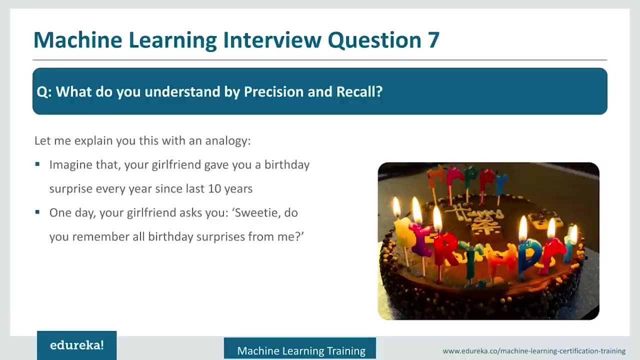 and you're just selecting the data from there. so in this case, you're getting bias to those conclusions of your- inaccurate conclusions of yours- and you're not making the accurate decisions based for the population. okay, so that is the selection bars. so what do you understand by precision and recall? so in this case, let's go on with the example. so let's imagine that 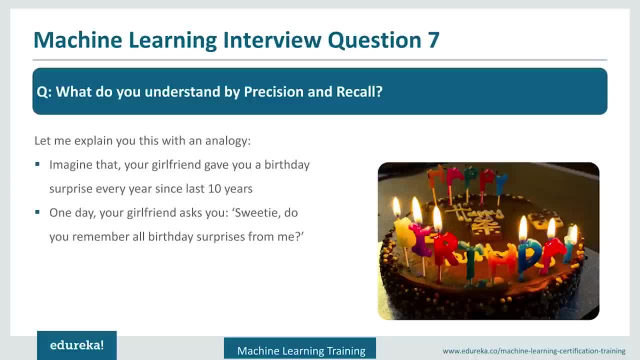 your girlfriend keep on giving you surprises from last 10 years of your birthdays and one sudden day she comes to you and asks you, do you remember all birthday surprises from me? and you just get shocked. and in this case, to extend your life. what you do is you try to understand the 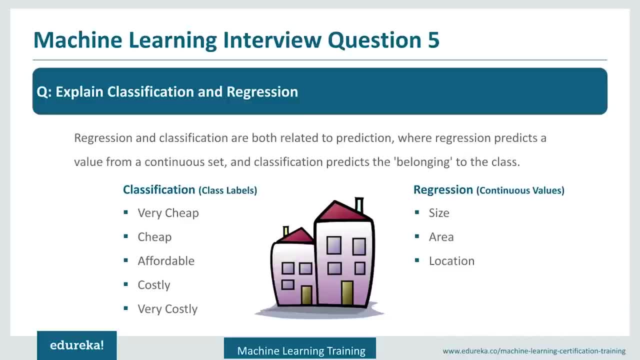 within the data. So, for example, the classes could be like: is the student going to pass or not, Is my customer going to buy my product or not, And is my salary is within like high, Medium, Low? So those are the different classes and when we're dealing with the classes, we say it. 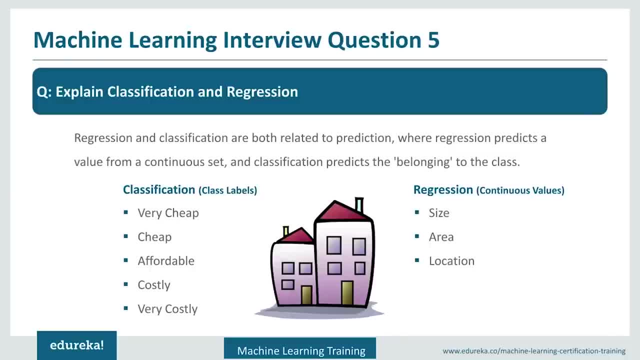 is classification and we're dealing with the continuous values. we say it is regression. So in this case, if you see, the regression is like size of your house area and the location which are there, and classification is like when you're trying to give it a classes. 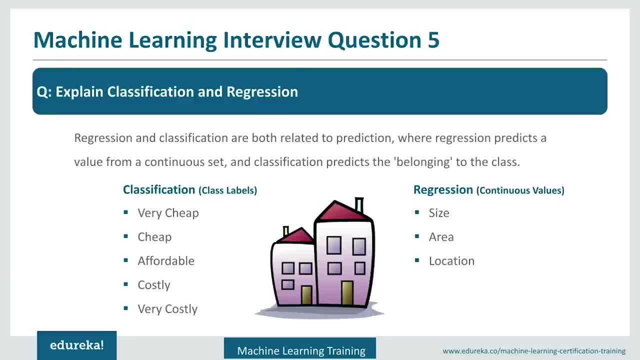 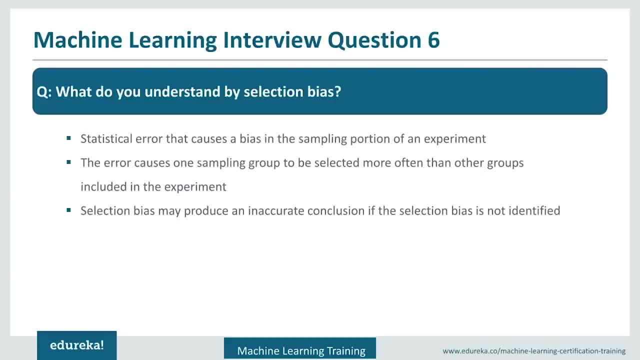 So very cheap, cheap, affordable. So you're creating a five classes here and that becomes a classification. What do you understand by selection In the statistical term? sampling is basically trying to sample some data from your population. So you are trying to take some portion of the data from the population and when you 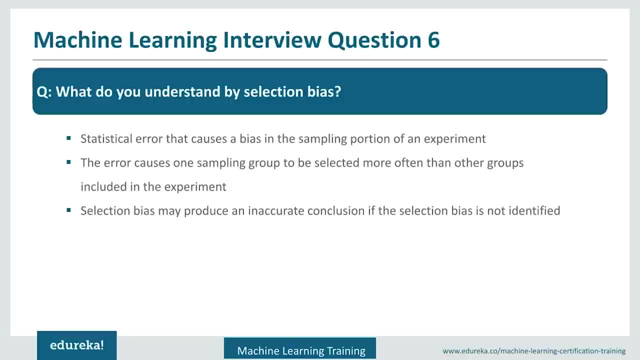 have some bias to some specific set of data. So let's assume we want to take a population of all the data scientists within India. When you're talking about India, you have to take data from all parts of India. but let's assume you just take the sample from the Gurgaon. 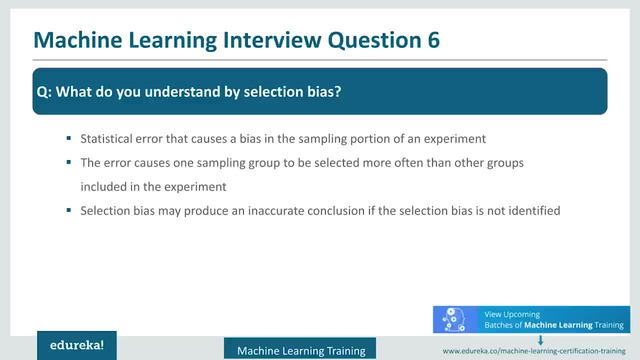 So when you just take the sample from the Gurgaon, you're getting a selection bias. You're getting bias to the Gurgaon and you're just selecting the data from there. So in this case you're getting bias to those conclusions of your inaccurate conclusions. 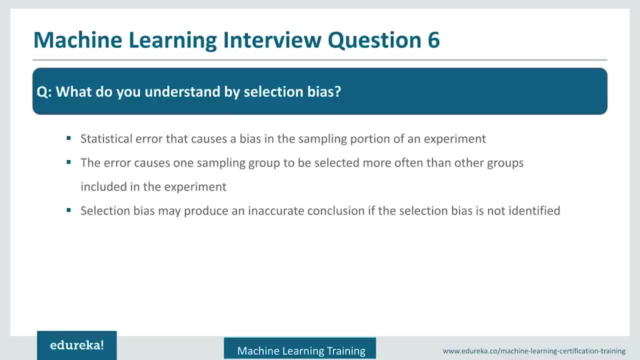 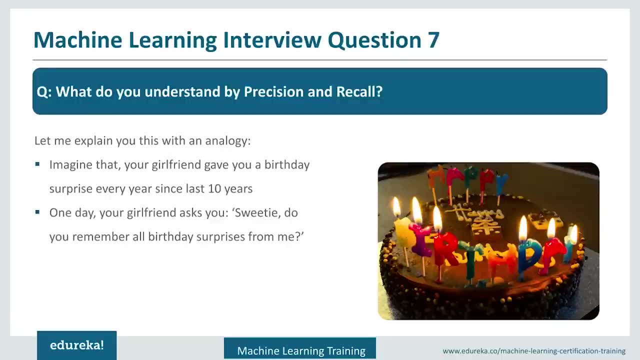 of yours and you're not making the accurate decisions based for the population. Okay, So that is the selection bias. So what do you understand by precision and recall? So in this case, let's go on with the example. So let's imagine. 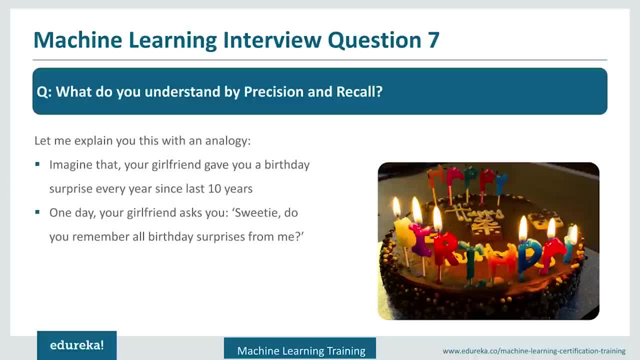 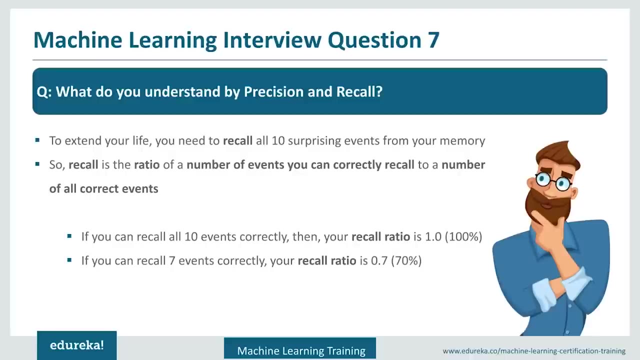 Imagine that your girlfriend keep on giving you surprises from last 10 years of your birthdays and one sudden day she comes to you and asks you: do you remember all birthday surprises from me? And you just get shocked. And in this case, to extend your life, what you do is you try to recall all the 10 surprising. 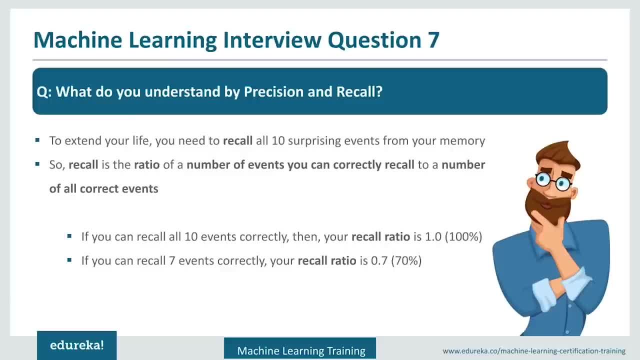 events that you had in your previous birthdays. And this recall that you're doing is nothing but the number of events you actually correctly trying to recall it And The number of events which have happened. So this is the ratio that you're trying to capture of all the recalls that you're doing. 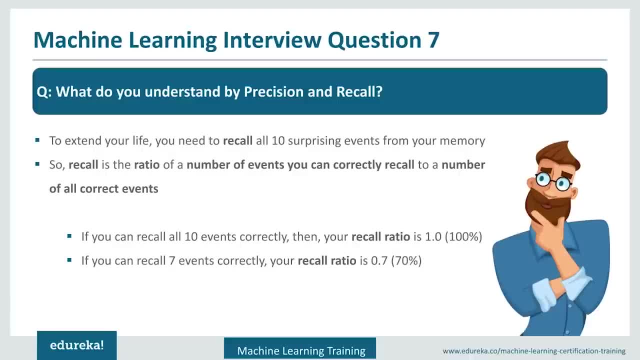 number of surprises from last 10 years and you try to recall all the 10 surprising events that you had in your previous birthdays. and this recall that you're doing is nothing but the number of events you actually correctly trying to recall it and the actual events which have happened. so this 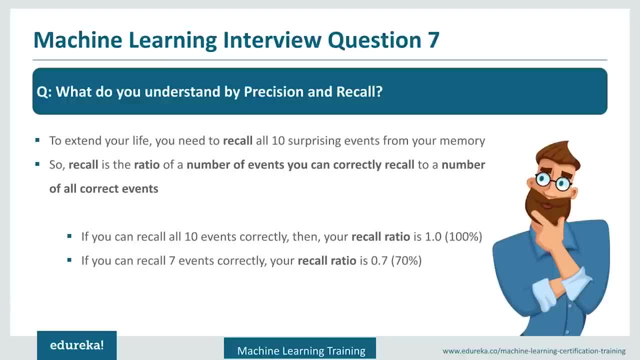 is the ratio that you're trying to capture of all the recalls that you're doing correctly and the number of the correct events which happened. so, for example, if you are trying to recall, out of 10, all but one, so which is again a hundred percent, but if you're trying to recall only seven events, 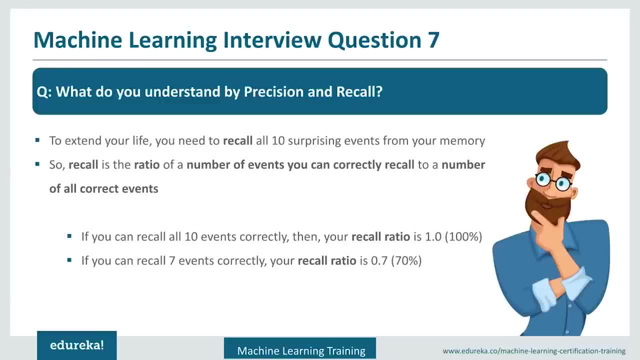 correctly. so, as per the ratio, what will happen is the number of events you can correctly recall is seven and the total number of events which are there is 10. so in this case your ratio will be 0.7, which will be 70 percent. but let's assume you might be wrong in some answers. 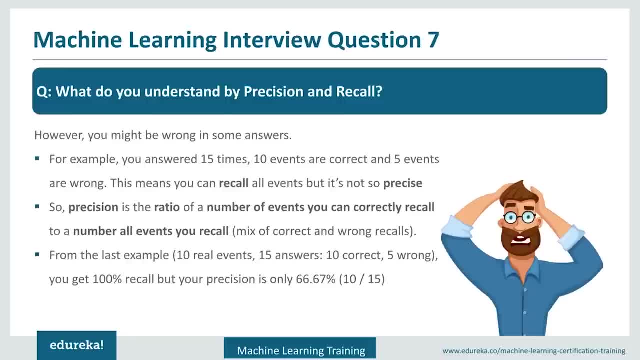 so, for example, you answered: you remember 15 times, but out of this only 10 were correct and five events were actually wrong. so you remembered from some another events. so in this case, so you recall all the events which are there, but it's not completely precise. so in this case, 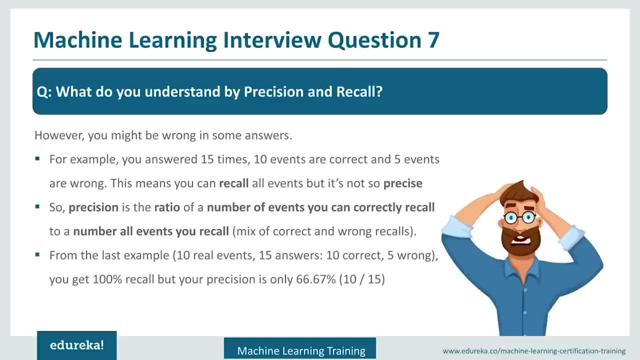 the precision is the ratio that the number of events you are recalling correctly to the number of events you recall. so which is like: out of 15, you are trying to recall the 10 as a character. so that is the precision which we have, so 10 real events and 15 answers. so the ratio is: 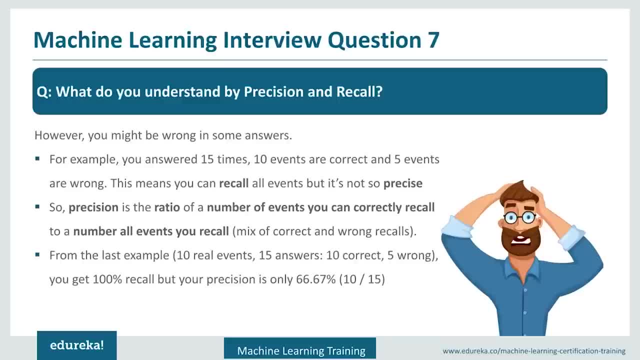 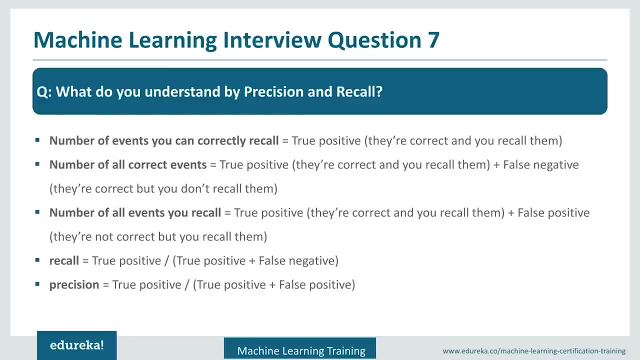 the 66 percent in this case, which is 10 divided by 15.. okay, in the formulas you can represent all those things in a simple formula. so number of events you can correctly recall are called as the true positive. so which you said as true, you said as a positive, you are able to recall them. 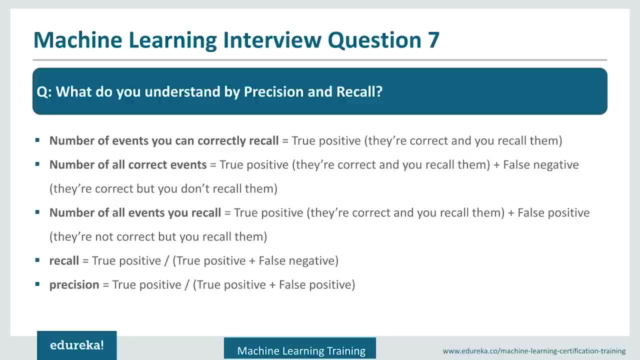 correctly and they are actually there. so, number of all correct events. so this is also again the true positive which you recall correctly, plus false negative which you didn't recall. okay, and the next thing is the number of events you recall, so which is true positives plus the false positives. in this case, what is happening? 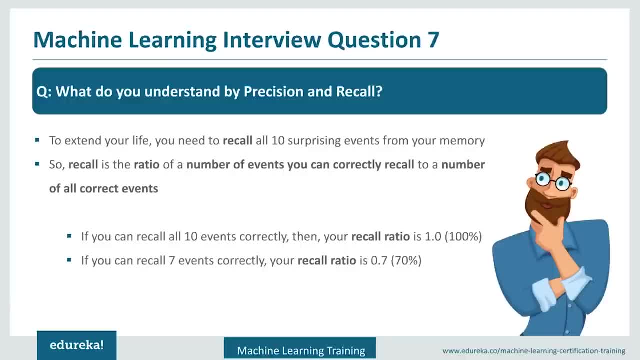 correctly and the number of the correct events which happened. So, for example, if you are trying to recall out of 10, all the 10 correctly, then your recall ratio is nothing but one, So which is again a hundred percent. But if you're trying to recall only seven events correctly, 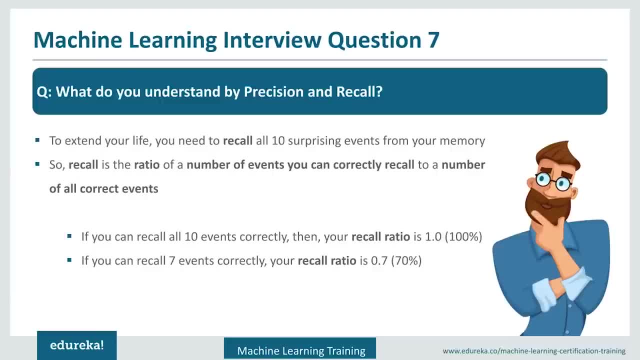 So, as per the ratio, what will happen is the number of events you can correctly recall is seven And The number of events which are there is 10.. So, in this case, your ratio will be 0.7, which will be 70%. 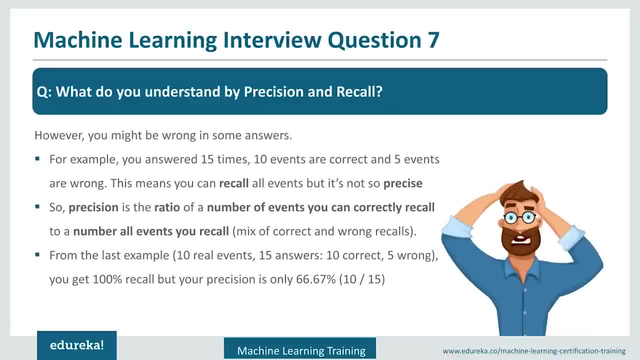 But let's assume you might be wrong in some answers. So, for example, you answered you remember 15 times, but out of this only 10 were correct and five events were actually wrong. So you remembered from some another events. So in this case, so you recall all the events which are there, but it's not completely precise. 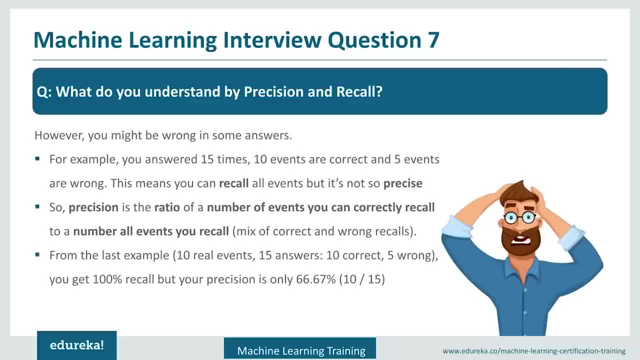 So in this case, the precision Is the ratio that the number of events you are recalling correctly to the number of events you recall. So which is like, out of 15, you're trying to recall the 10 as a character. So that is the precision which we have. 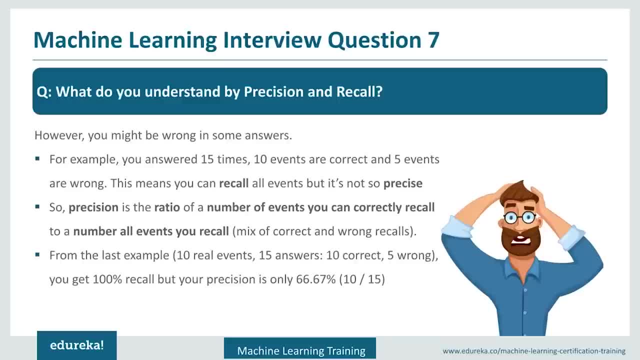 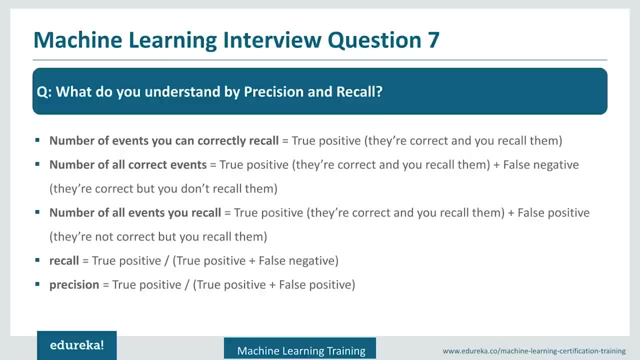 So 10 real events and 15 answers. So the ratio is the 66% in this case, which is 10 divided by 15.. Okay, In a formula, you can represent all those things in a simple formula. So number of events you can correctly recall. 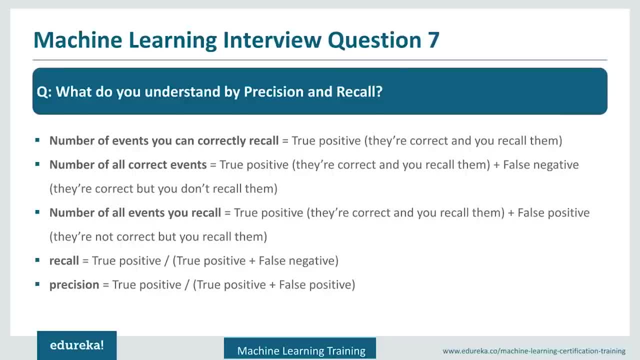 So all the positive and negative events are called as the true positive. So which you said as true, you said as a positive, you are able to recall them correctly and they're actually there. So number of all correct events. So this is also again the true positive which you recall correctly. 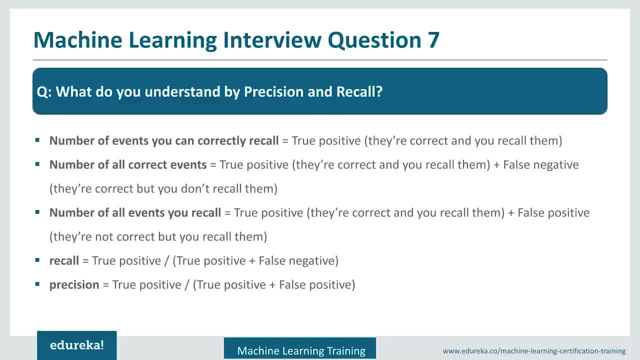 Plus the false negative which you didn't recall. Okay, And the next thing is the number of events you recall. So which is true positives plus the false positives? In this case, what is happening is the correct recall that you did, all the events that you. 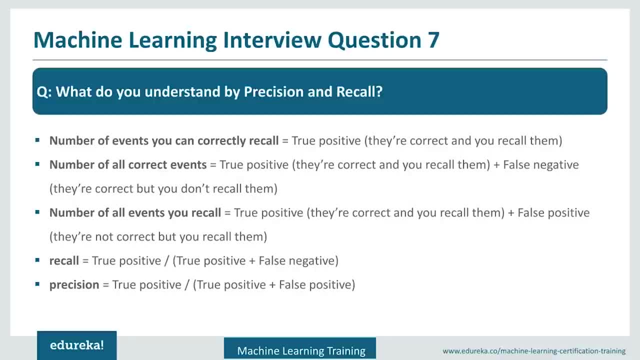 correctly remembered and some which are not correct. So you said: okay, I recall them. So, for example, when we had it 15, so in that case there were some like 10 were correct and five were the false positive, which was, you didn't recall them correctly. 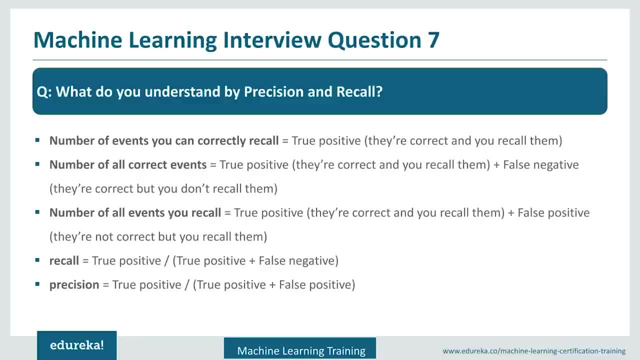 is the correct recall that you did, all the events that you correctly remembered and some which are not correct. so you said, okay, i recall them. so, for example, when we had it 15, so in that case there were some like 10 were correct and 5 were the false positive. 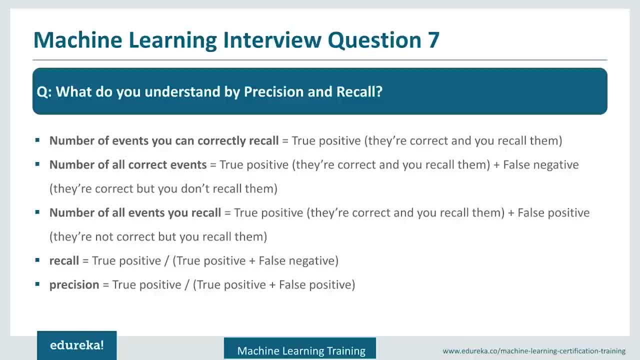 which was you didn't recall them correctly. so, based on all this above recall is true positive divided by true positive plus false negative. so true positive plus false negative is nothing but the number of correct events, as we already saw that. so number of events you can correctly recall. 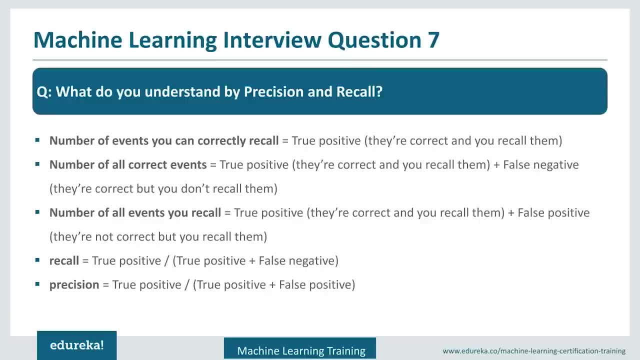 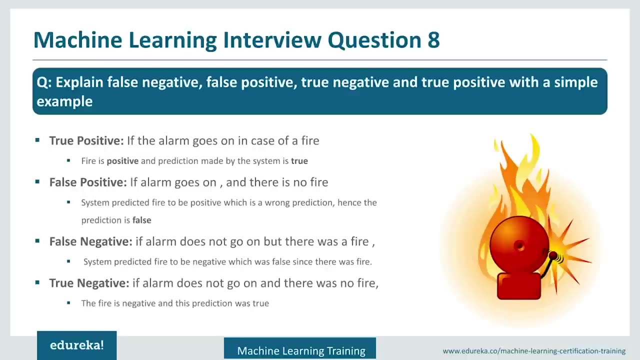 divided by number of correct events and precision, is true positive divided by true positive plus false positive, which is the number of events you can correctly recall divided by number of all events you recall. okay, so the next question is explain false negative, false positive, true negative and true positive with a simple example. so previously we just saw the example. 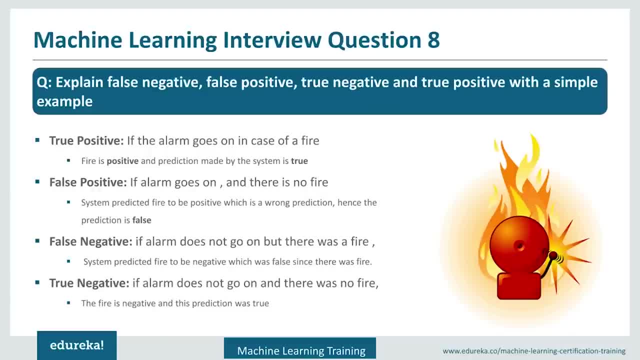 where we had an example of the birthday surprises. so you can also go with the example where it will be more realistic as it will give some impact to it. so, for example, the true positive. so in this case we can take some real example where what the model that we are trying to build, what it does. 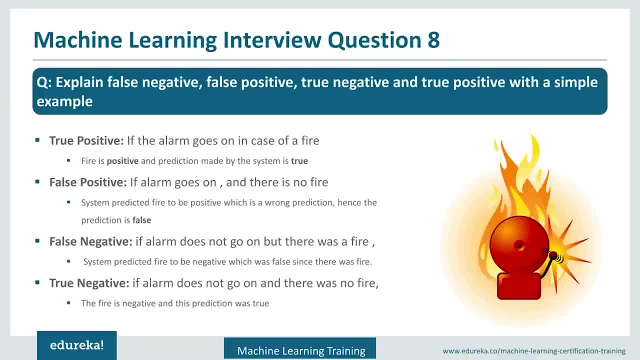 is based on the fire is there or not, it will try to raise an alarm. so in the first case, it's true, positive. so in true positive, what will happen is: you said you have to do the alarm and there is actually a fire, so there is actual fire and you try to do it. it is the right condition. 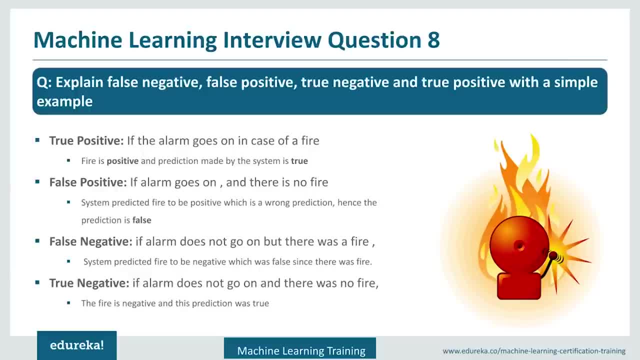 so that is the true positive. second is the false positive. in this case, you raise an alarm but there is no fire. so in this case, what will happen? when you raise the alarm, there is no fire but still people are running. so that is not a good thing and that is called the false positive. 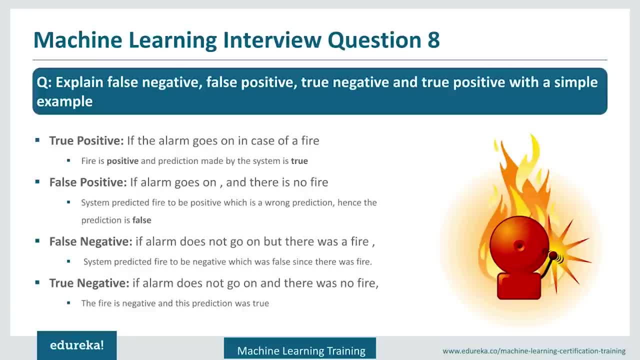 third example is false negative. so false negative. if you are not raising an alarm, even when there is a fire. this is the worst condition that we have in all the situations. so your aim is to raise an alarm when there is actual fire, but this condition says, when you there is still a fire, you are not. 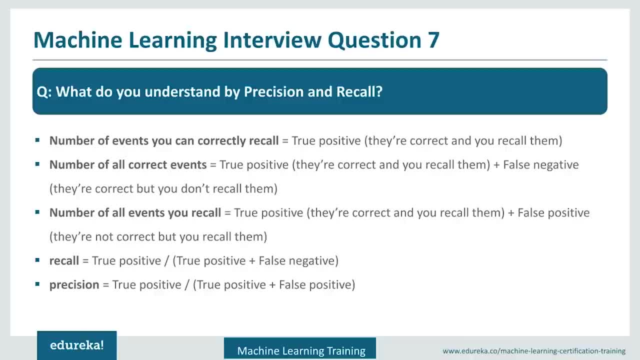 So, based on all this above, recall is true positive divided by true positive plus false negative. So true positive plus false negative is nothing, Okay, Nothing but the number of correct events, as we already saw that. So number of events you can correctly recall divided by number of correct events and precision. 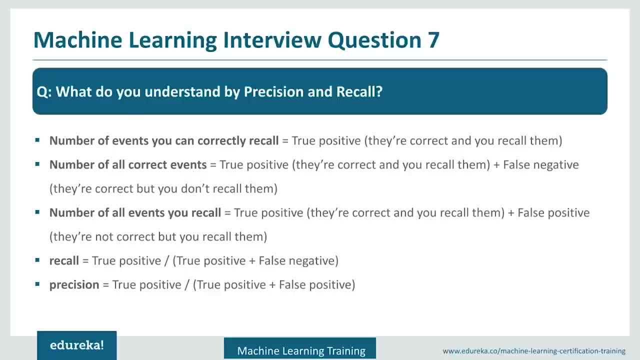 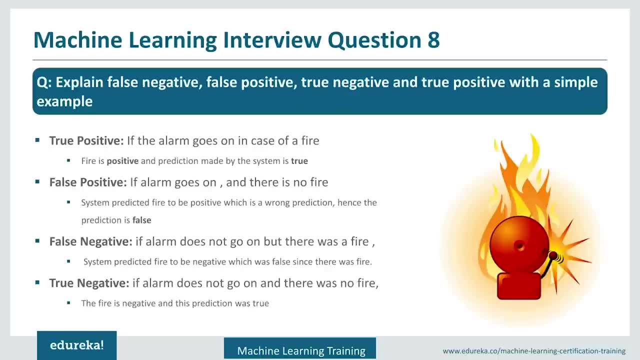 is true positive divided by true positive plus false positive, which is the number of events you can correctly recall divided by number of all events you recall. Okay, So the next question is explain false negative, false positive, true negative and true positive with a simple example. 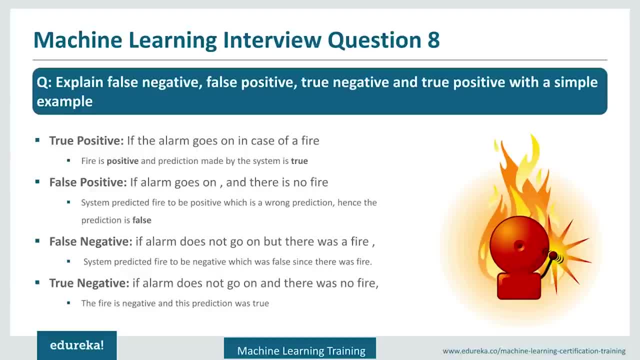 So previously we just saw the example, We had an example of the birthday surprises. so you can also go with the example where it will be more realistic as it will use an impact to it. So, for example, the true positive. So in this case we can take some real example where what the model that we are trying to 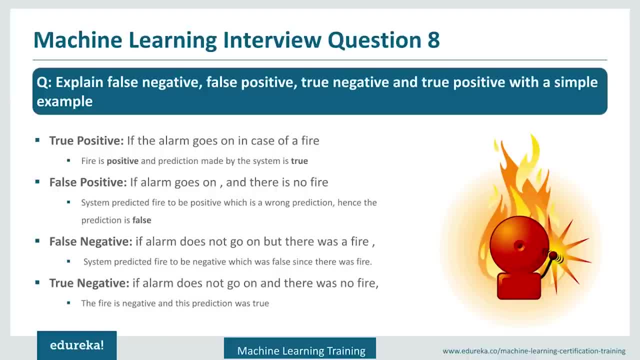 build. what it does is based on the fire is there or not. it will try to raise an alarm. So the first case, it's true positive. So in true positive, what will happen is: you said You have to do the alarm and there is actually a fire. 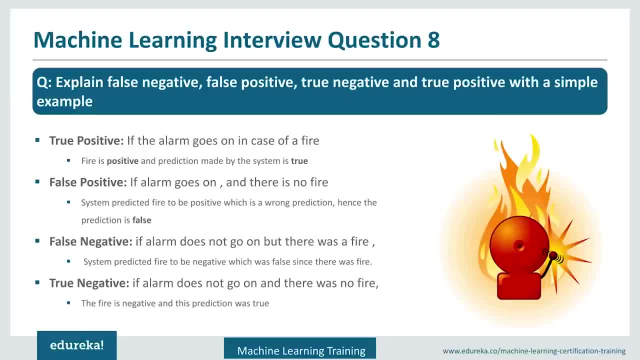 So there is actual fire and you try to do it. It is the right condition. So that is the true positive. Second is the false positive. In this case you raise an alarm, but there is no fire. So in this case, what will happen when you raise the alarm? there is no fire, but still. 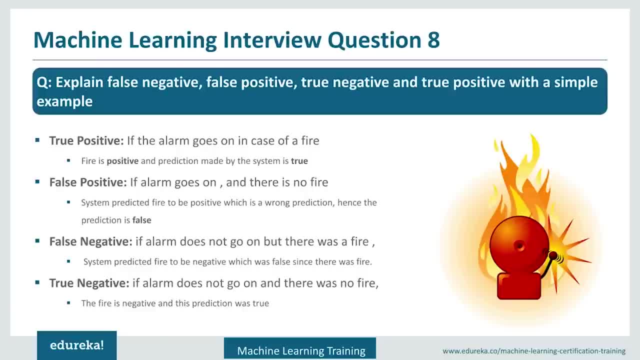 people are running, So that is not a good thing And that is called the false positive. Third example is false negative, So false negative If you're not raising an alarm, even when there is a fire. this is the worst condition that we have in all the situations. 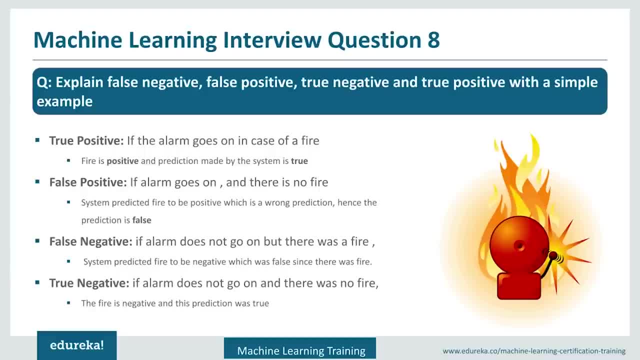 So your aim is to raise an alarm when there is actual fire, But this condition says: when there is still a fire, you're not raising any alarm. So this is the most harmful thing which can be there and where your model is not working. 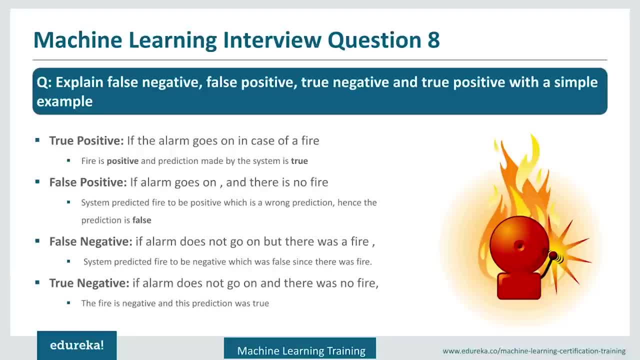 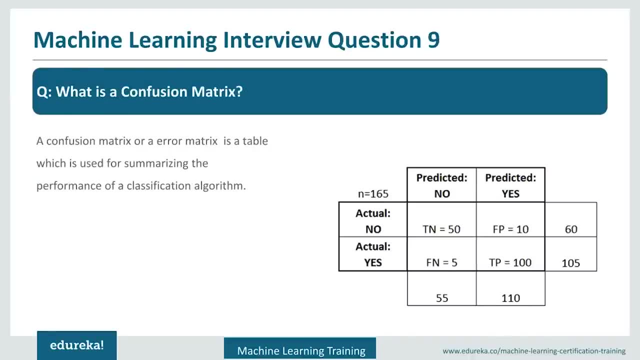 So you have to be very careful with this thing. one And true negative is something where there is no fire and you have not raised any alarm, which is still false. This situation is a very good example. Okay, What is confusion matrix? So to explain this confusion matrix to your interview, you can take some simple examples. 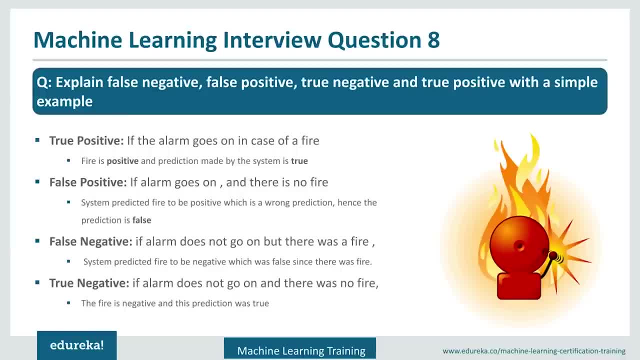 raising any alarm. so this is the most harmful thing which can be there and where your model is not working. so you have to be very careful with this thing. one and true negative is something where there is no fire and you have not raised any alarm, which is 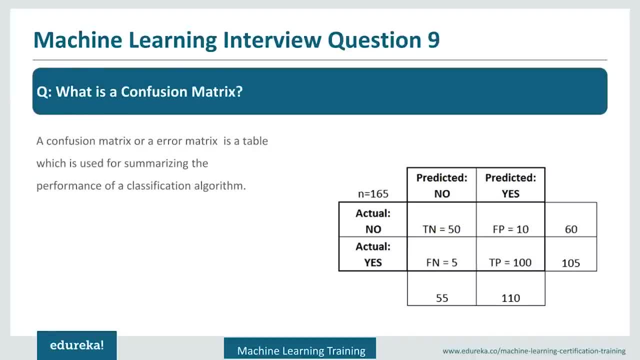 still good. okay, what is confusion matrix? so to explain this confusion matrix to your interview, you can take some simple examples, such as: you want to create a model where what you are trying to look is you have a bank and that bank wants to identify who are the customers. i should be. 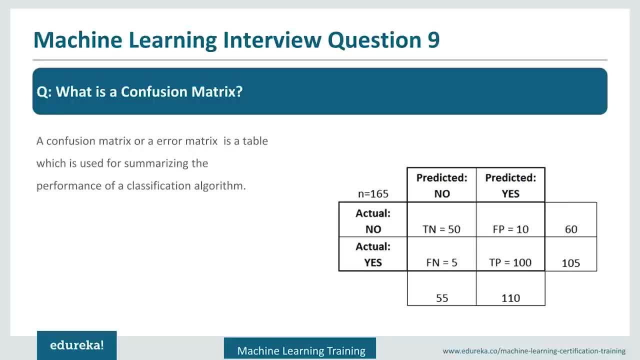 giving loan to so that they won't default me. so i have a training data where i know that, okay, these are the customers who were good, who didn't default, and these are the customers to whom i gave loan but they defaulted. so that data is used in making these predictions and you have a model which has 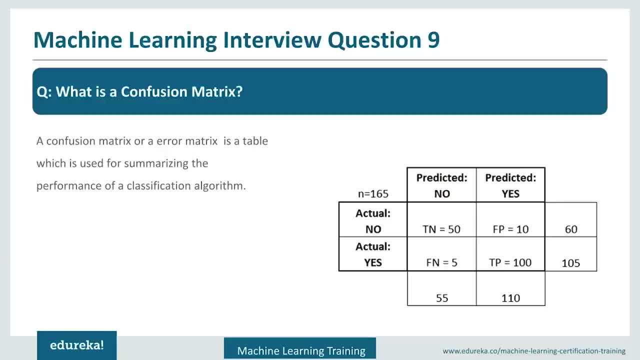 done this also. so assume that we have 165 people in the training set and after doing the prediction, so in the training set what we have got is, in actual, hundred and five people can be given loan defaulted and 60 people who bank gave loan they defaulted. so what your model is predicting in. 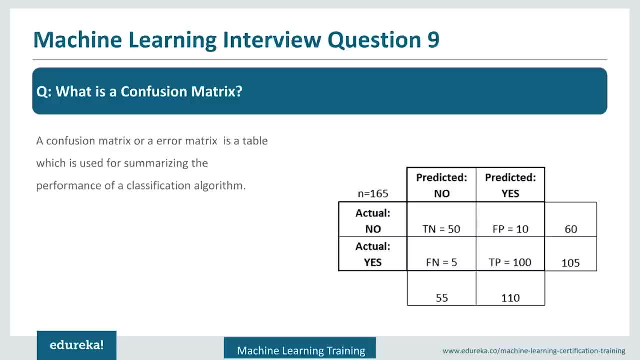 this case is. it says 110 people can be given loan who will not default and 55 people can be rejected. so as they are going to default, but this is on a higher level. but when you look as a confusion matrix, what will happen is you will try to see, okay, how my model is performing and where. 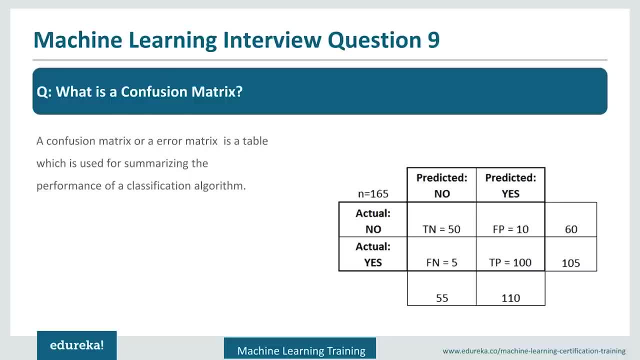 are the true positives, true negatives, and how should i take care? uh, not take care, but how is it performing at the part of the false positive and the false negatives? so assume we have a true positive. so in actual there are 105 people who are the bank's training data says can be given. 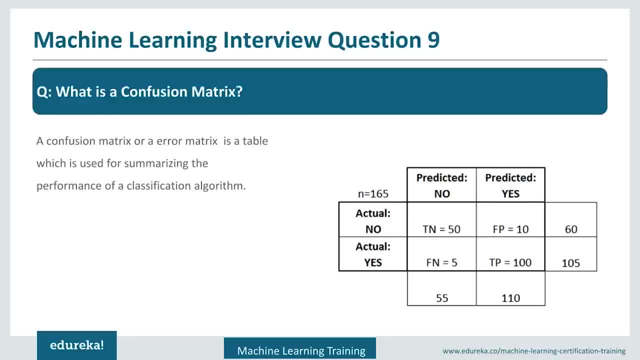 loan who didn't default. but out of that model has identified 100 people, so, which is a good thing. and for the no case, for the rejection case, out of 60 people, the model says 50, which is again a good thing. but your model says: for 10 people who are actually defaulters, 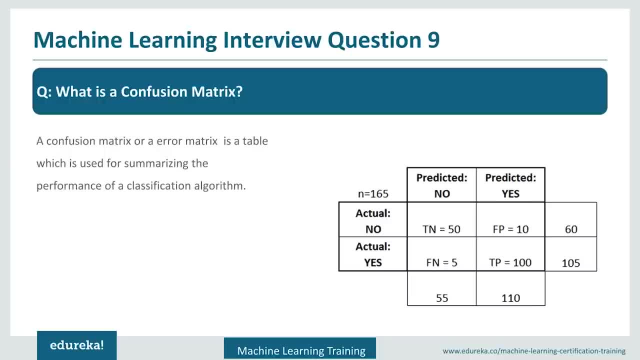 such as if you want to create a model of what you're trying to look is you have a bank and that bank wants to identify who are the customers I should be giving loan to so that they won't default me. So I have a training data where I know that, okay, these are the customers who were good. 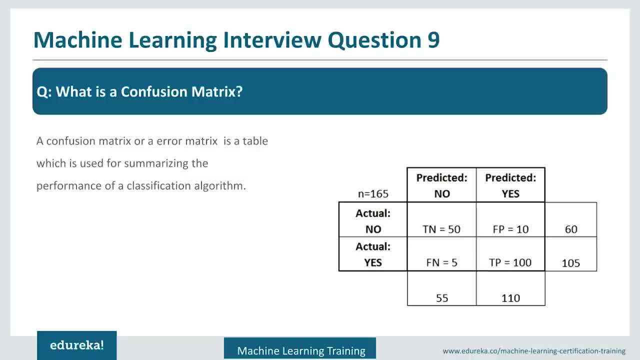 who didn't default, And these are the customers whom i gave loan but they defaulted. so that data is used in making these predictions and you have a model which has done this also. so assume that we have 165 people in the training set and after. 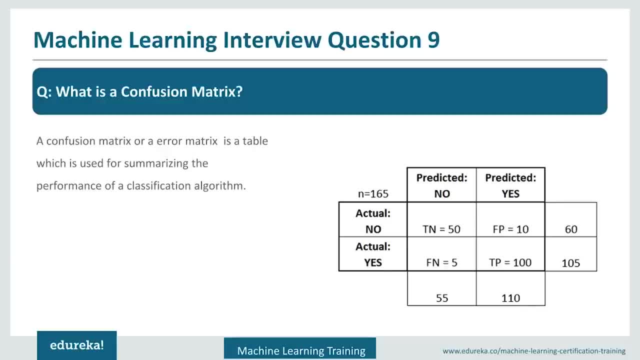 doing the prediction. so in the training set, what we have got is, in actual, 105 people can be given loan who didn't defaulted and 60 people who bank gave loan they defaulted. so what your model is predicting in this case is it says 110 people can be given loan who will not default and 55 people 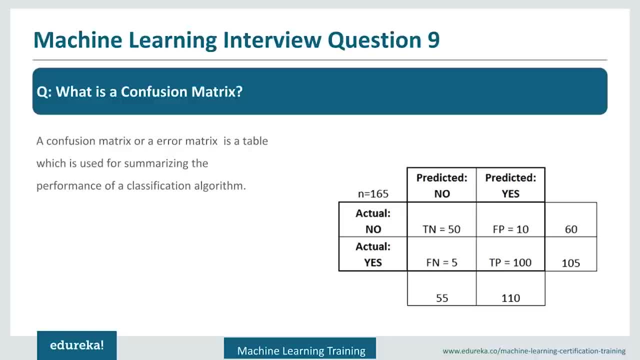 can be rejected, so, as they are going to default, but this is on a higher level. but when you look at the confusion matrix, what will happen is you will try to see, okay, how my model is performing and where are the true positives, true negatives, and how should i take care? uh, not take care, but 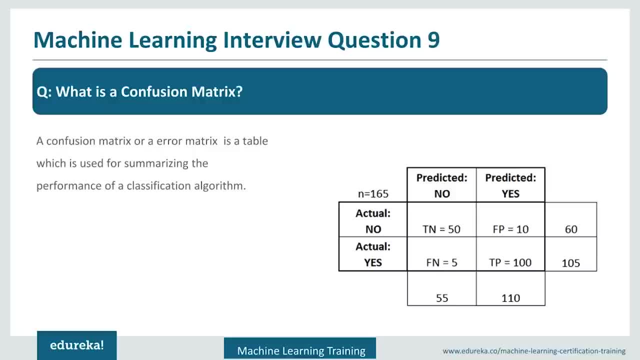 how is it performing at the part of the false positive and the false negative? so assume we have a true positive, so in actual there is a true positive and there is a false negative, so in actual there is a true positive. there are 105 people who are the banks training data says can be given loan who didn't default. 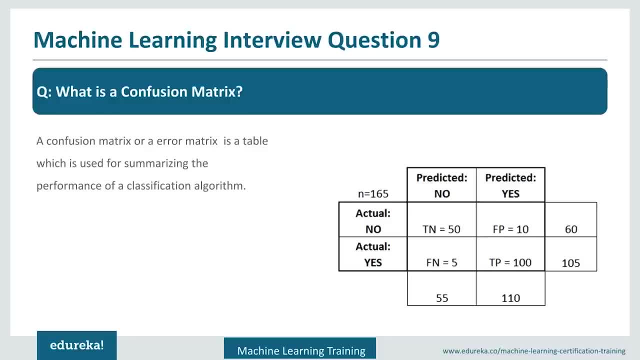 but out of that model has identified 100 people, so which is a good thing. and for the no case, for the rejection case, out of sixty people, the model says fifty, which is again a good thing. but your model says for ten people who are actually defaulters, but model says you should. 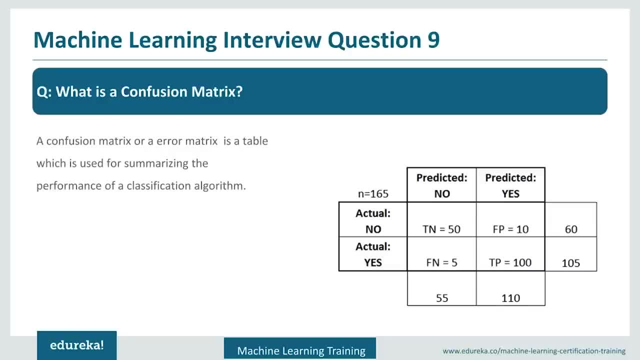 give them loan. so those are the things which can be looked into the future, but confusion matrix will help you to understand how your model is performing, based on the predicted, the model output and the actual data which you have. So what is the difference between inductive? 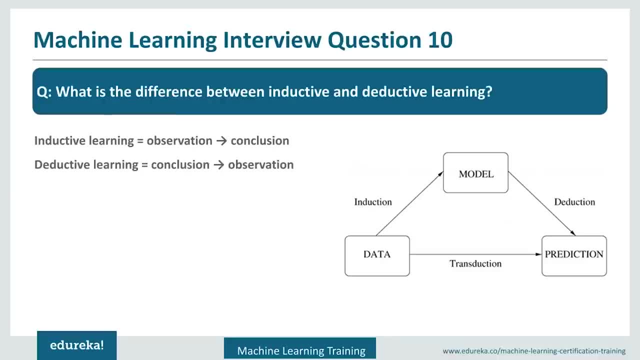 and deductive learning. So to help this concept, you can give some good examples, such as a father want to explain his son how the fire can burn him. So there are two ways that he can teach his kid how he can get impacted from the fire. So first thing is he will show him some examples. 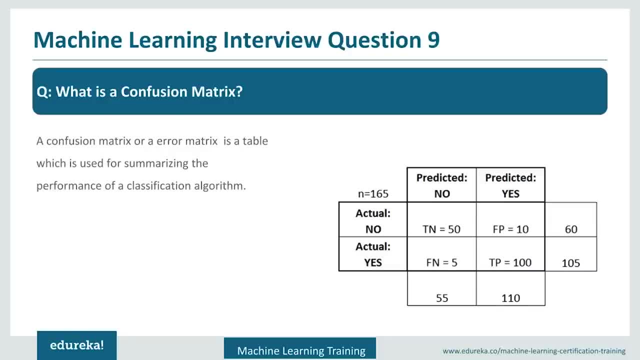 but model says you should give them loan. so those are the things which can be looked into the future, but confusion matrix will help you to understand how your model is performing, based on the predicted, the model output and the actual data which you have. so what is the difference between 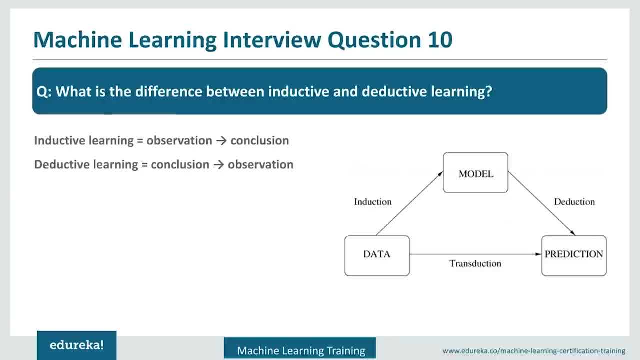 inductive and deductive learning. so to help this concept, you can give some good examples, such as a father want to explain his son how the fire can burn him, so there are two ways that he can teach you how to explain his son how the fire can burn him. so there are two ways that he can teach you. 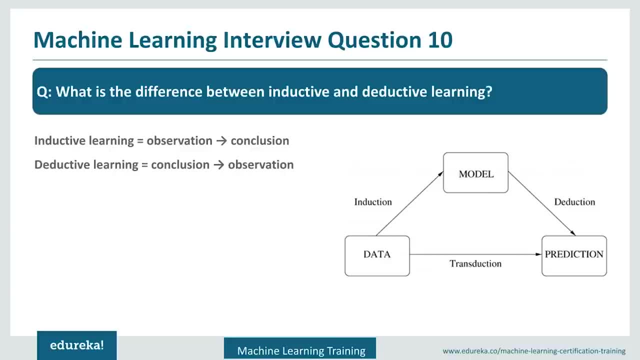 kid as how he can get impacted from the fire. so first thing is he will show him some examples, like he will show him some videos or he will show some demo as how the fire will get him burned. so, based on the observations, the kid will learn and make some conclusions out of it. so that is. 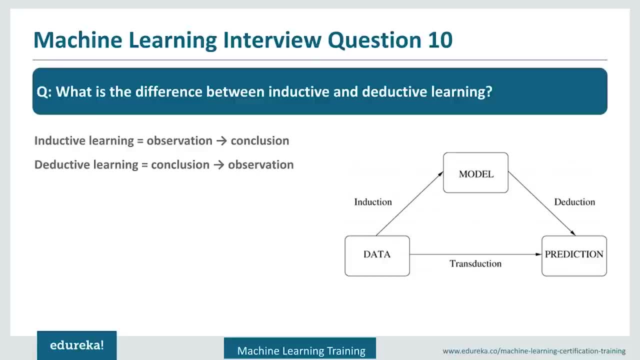 the example for inductive of learning, where he will do the observation and see how the things are going to be and make some conclusions out of it, and for the deductive learning it is like father is letting the kid play with the fire, so the father will wait till kid will get burned and 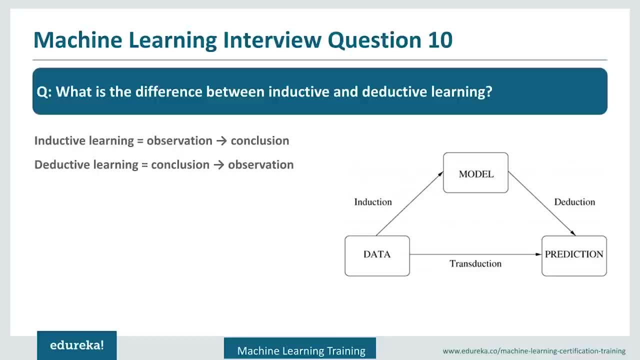 try to make some conclusions out of it and have the observations after it, like he will get himself burned and then he will say that okay, fire makes us burn. so that is the deductive learning, where what happens is: first you will make some conclusions and then you draw the observations. similarly in the 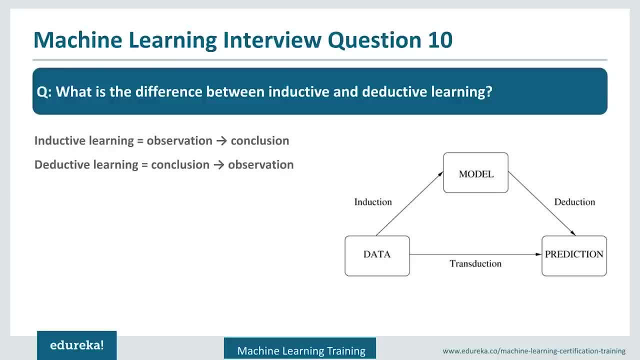 field of machine learning. it is like, out of the data, you will try to do some observations and this is the way that the observations are stored as a model, which is like you have observed all the things and kept it as a model. and the deductive learning is like you are giving it a data and 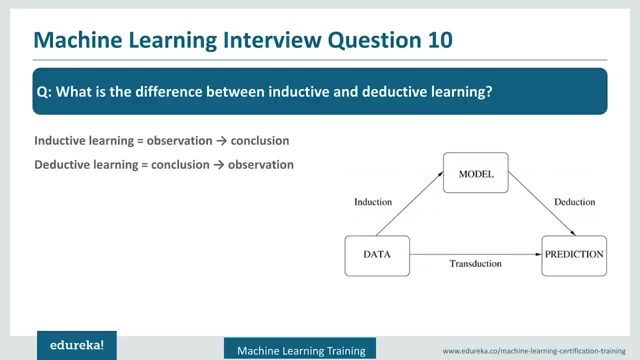 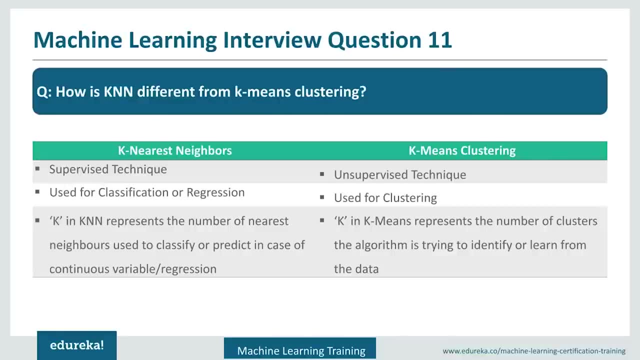 based on the previous inductive learning that it has already done, it will try to deduce the output of it. so how is knn different from k-means clustering? one important thing happens is people are really confused with what is knn, or sometimes like: is knn clustering, or if k-means are. 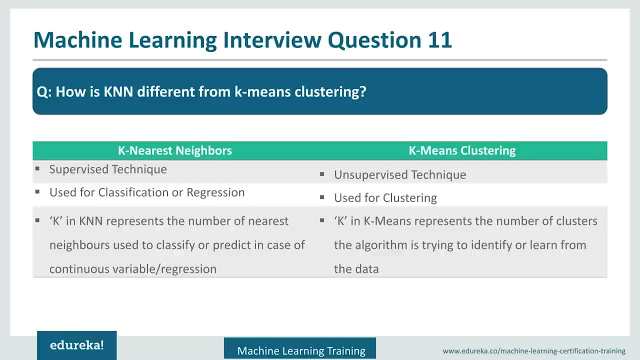 clustering. in this question, the clustering is given to you as a model and you have to learn it. as k-means clustering, but sometimes the integral, just ask you: how is knn different from k-means? first thing you have to do is you have to understand the difference, as k-means is. 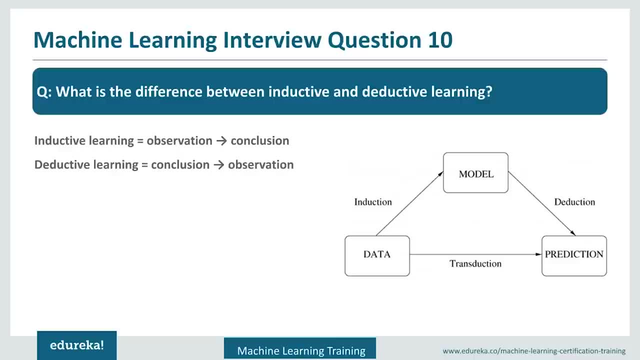 Like he will show him some videos or he will show some demo as how the fire will get him burned. So based on the observations, the kid will learn and make some conclusions out of it. So that is the example for inductive learning, where he will do the observation and see how the things are going. 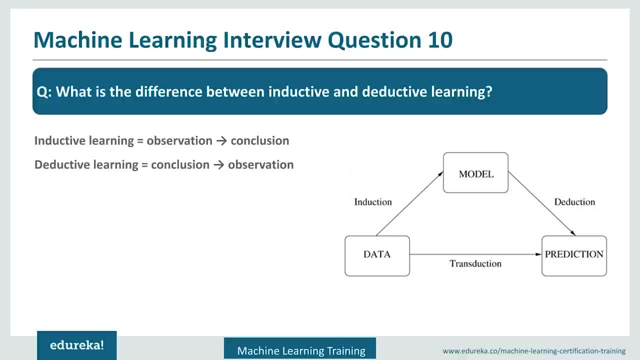 to be and make some conclusions out of it And for the deductive learning. it is like father is letting the kid play with the fire, So the father will wait till kid will get burned and try to make some conclusions out of it and have the observations after it Like he will get himself. 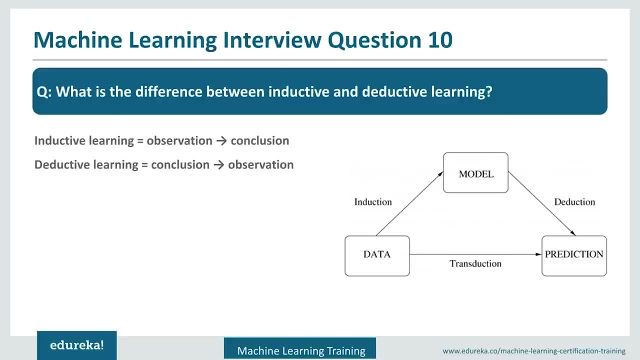 burned and then he will say that okay, fire makes us burn. So that is the deductive learning, where what happens is: first you will make some conclusions and then you draw the observations. Similarly, in the field of machine learning, it is like: out of the data, you will try to do some observations. 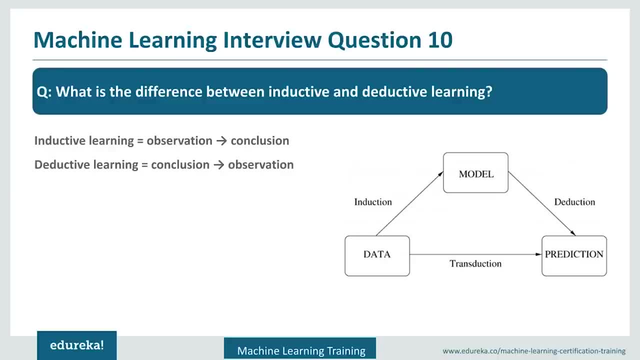 and these observations are stored as a model, which is like you have observed all the things. the deductive learning is like: you are giving it a data and, based on the previous inductive learning that it has already done, it will try to deduce the output of it. So how is KNN different from K-means? 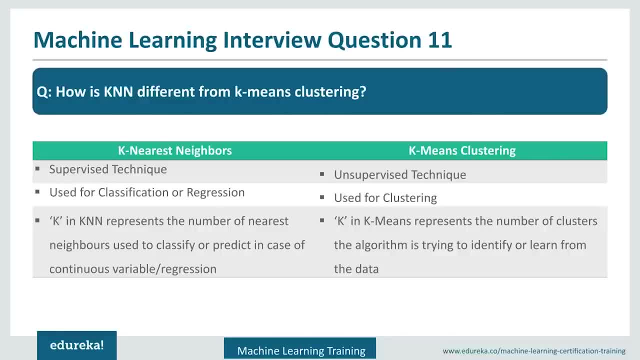 clustering. One important thing happens is people are really confused with what is KNN or sometimes like: is KNN clustering or is K-means a clustering? In this question, the clustering is given to you as K-means clustering, but sometimes the intern will just ask you: how is KNN different from K-means? 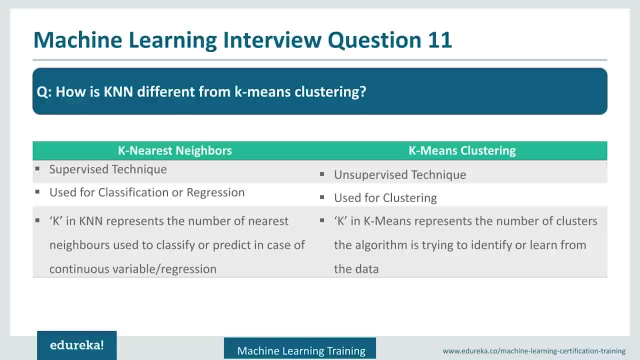 The first thing you have to do is you have to understand the difference, as K-means is an unsupervised technical algorithm and KNN is a supervised technique In. KNN is used as a supervised algorithm, KNN is used for classification, regression, and K-means is used for clustering. as it is a clustering, 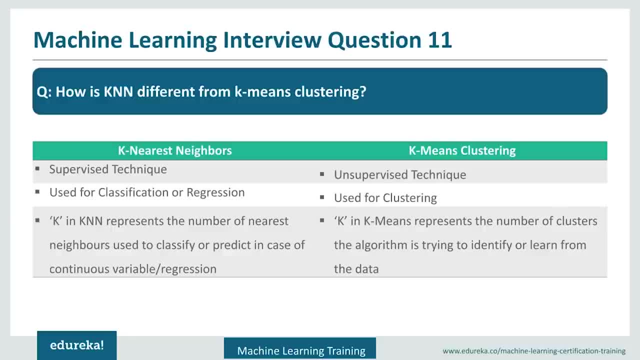 algorithm it is used to do create the clusters of your data. K within KNN basically means it tries to observe the KN neighbors. So in the case of regression, it will try to identify the surrounding K neighbors and take the average and give you the output. and in the case of classification, what it will do is it will 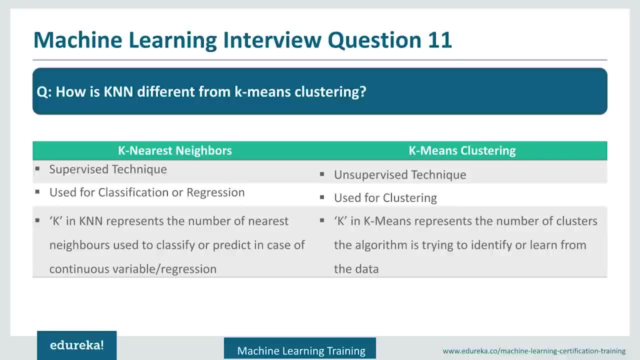 a unsupervised technique algorithm and knn is a supervised technique and knn is used as a supervised algorithm. knn is used for classification, regression and k-means is used for clustering. as it's a clustering algorithm, it is used to do create the clusters of your data. 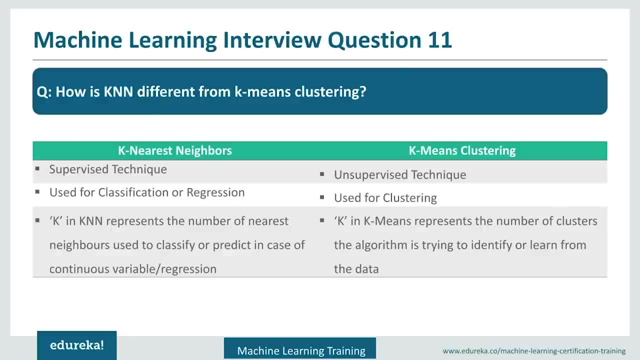 k within knn basically means it tries to observe the k neighbors. so in the case of regression, it will try to identify the surrounding k neighbors and take the average and give you the output. and in the case of classification, what it will do is it will try to see the surrounding. 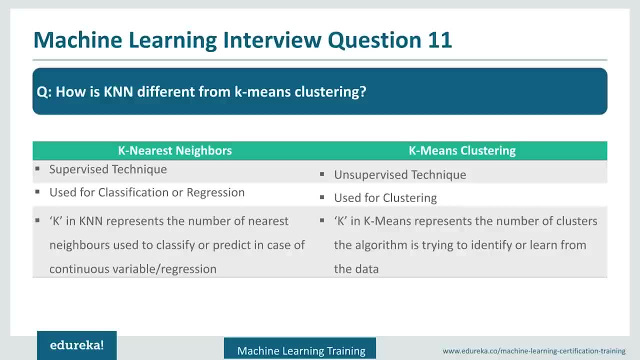 neighbors, k neighbors, and whatever the majority of the class is there, it will assign the class to that. so, in this case, k is your neighbors, based on which your regression and classification will be done. in the case of k-means, it is the k clusters that you are going to create out of your data. 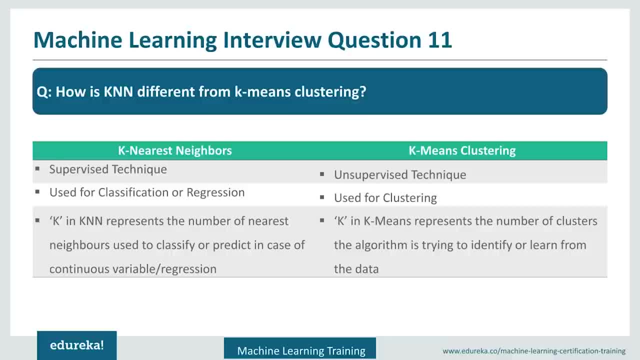 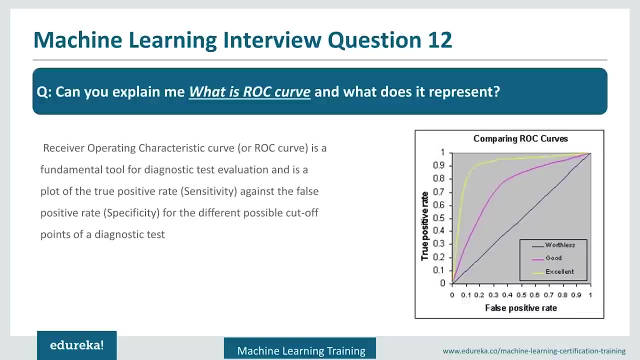 so k in the both cases is different and you have to give this differences to the interviewer. so one thing is you, once you know that, okay, k-means is an unsupervised and knn is a supervised, you can further go on top of that. okay, can you explain me what is roc curve and what does that represent? 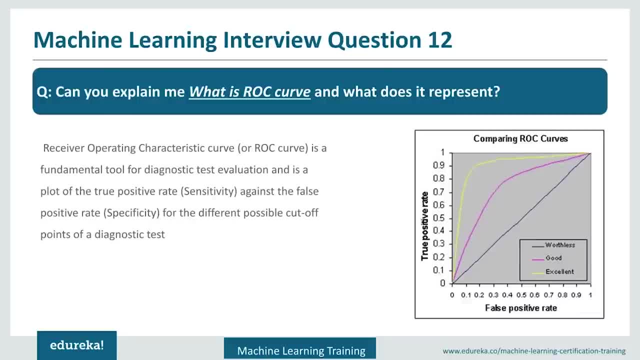 so in this case, interviewer is interested to know how good you understand the roc curve and how you can use it to understand your model's output. so inter is very much interested as how you are trying to use this in your model performance. so as roc is also one of 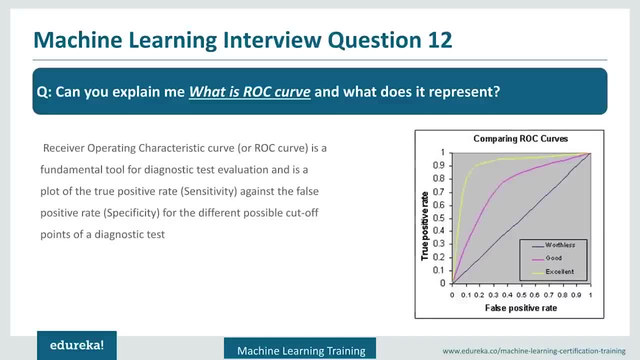 the performance parameters for your model and this is used in the cases of binary classification. the full form for the roc is receiver operating characteristics curve and its fundamental use started with the diagnostic test evaluations. so in the medical field its application started and it is used in the machine learning field to 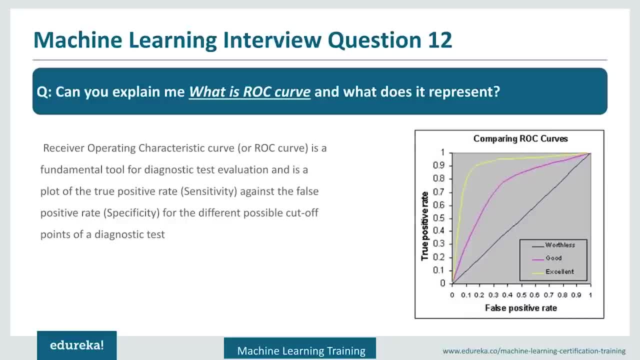 do the classification related algorithms, performance evaluation. so in simplistic term, it is the plot of true positive rates, which is also called as the sensitivity against the false positive rate. so what happens is, once you get the output in the probabilities, you can use the different cutoffs and you can use the cutoffs to distinguish as what is going to be the true cases. 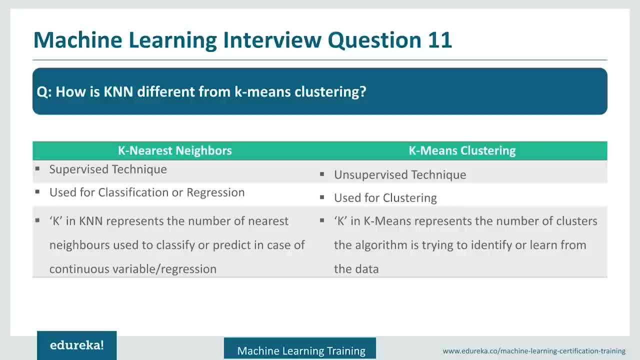 try to see the surrounding neighbors, K neighbors- and whatever the majority of the class is there, it will assign the class to that. So, in this case, K is your neighbors, based on which your regression and classification will be done. In the case of K-means, it is the K clusters that you are going to create out of your data. 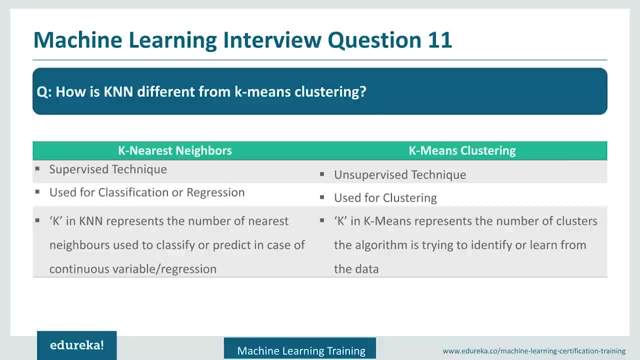 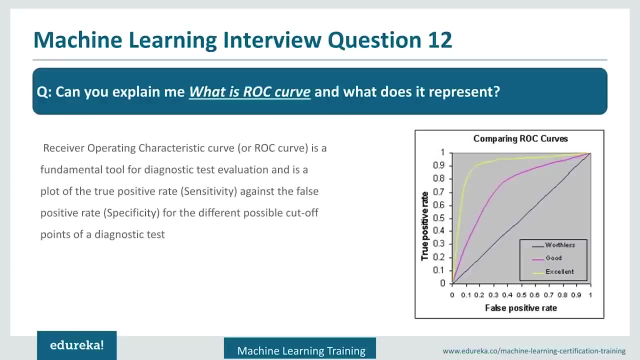 So K in the both cases is different and you have to give this differences to the interviewer. So one thing is you, once you know that, okay, K-means is an unsupervised and KNN is a supervised, you can further go on top of that. okay, Can you explain me what is ROC curve and what? 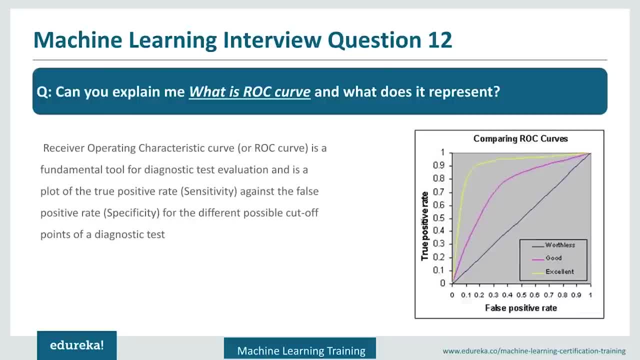 does that represent? So in this case, interviewer is interested to know how good you understand the ROC curve and how you can use it to understand your models output. And interviewer is very much interested as how you are trying to use this in your model performance. So as ROC is also one of the performance parameters for your model. 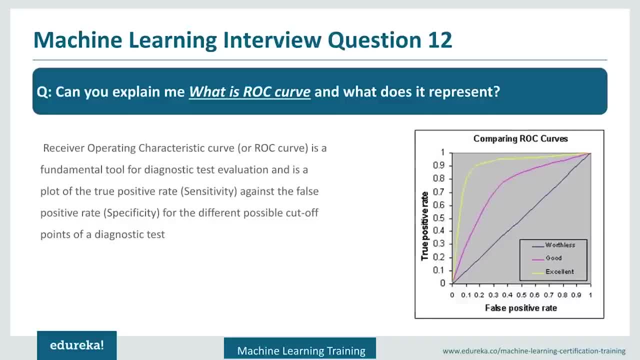 and this is used in the cases of binary classification. The full form part, the ROC, is receiver operating characteristics curve and its fundamental use started with the diagnostic test evaluations. So in the medical field its application started and it is used in the machine learning field to do the classification. 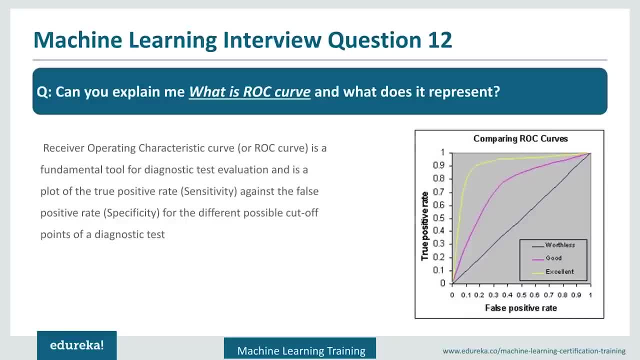 classification related algorithms, performance evaluation. so in simplistic term, it is the plot of true positive rates, which is also called as the sensitivity against the false positive rate. so what happens is, once you get the output in the probabilities, you can use the different cutoffs, and you can use the cutoffs to distinguish as what is going to be the true cases and what is. 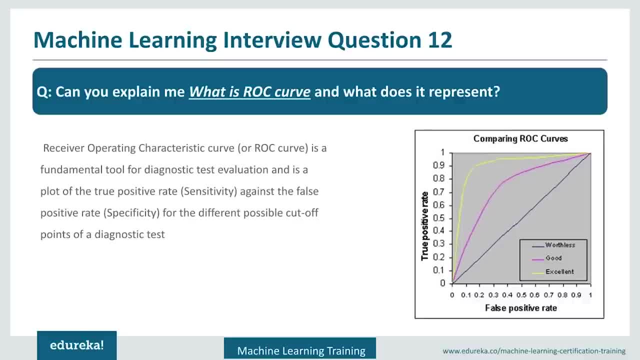 going to go for a false cases and you can plot the ROC curve and ROC curve says: when your curve is having one, your model is good and the plot with the 50 percent like 0.5, which is nothing but this blue line which is the worst case. it's like your model is saying you have a 50 percent chance in. 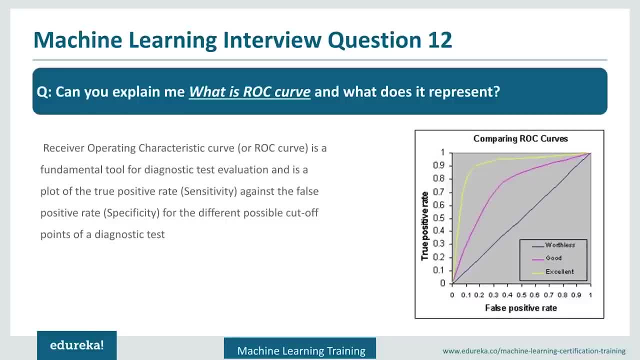 the prediction. it's just saying it's just a normal guessing work, so you're either guessing one or two with a 50 percent probability. the more closer to this and more area this curve is trying to cover, you're going to get a false case. and you're going to get a false case and you're going to get a. 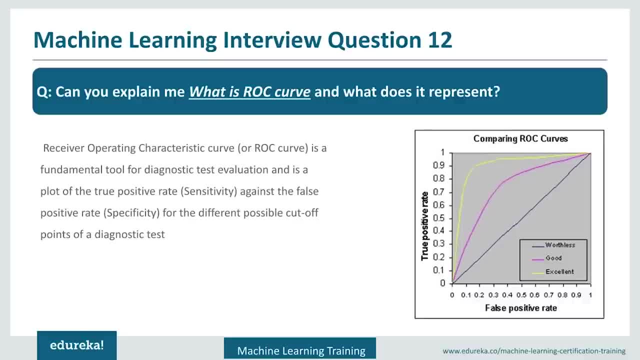 and what is going to go for a false cases and you can plot the roc curve and roc curve says: when your curve is having one, your model is good and the plot with the 50 percent like 0.5, which is nothing but this blue line, which is the worst case. it's like your model is saying you have a 50 percent. 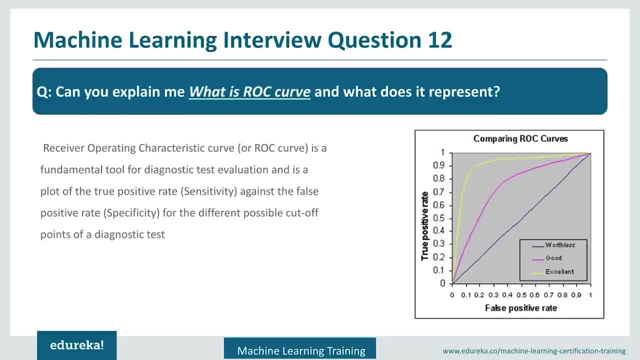 chance in the prediction it's just saying it's just a normal guessing work. so you're either guessing one or two with a 50 probability. the more closer to this and more area this curve is trying to cover, the better is the algorithm, so better you are trying to predict the true positive rates. 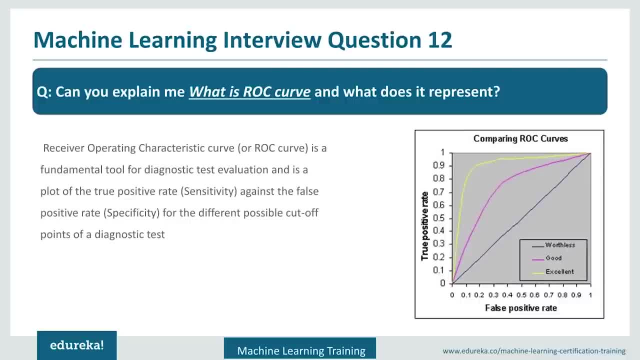 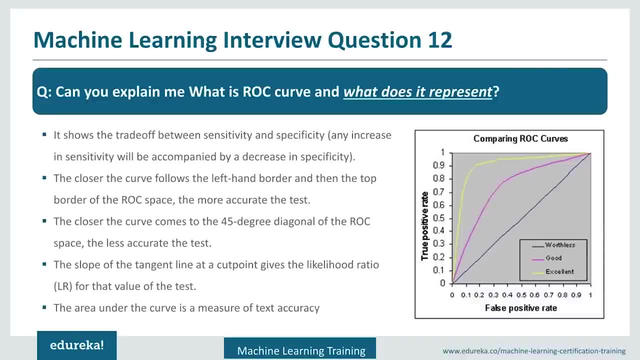 than the false negative rates. your true positive rate should increase faster than the false positive rates in this case. so first we saw like what actually roc curve does and we will see like how you can interpret it now so you can give the interview some idea about what is really roc curve. 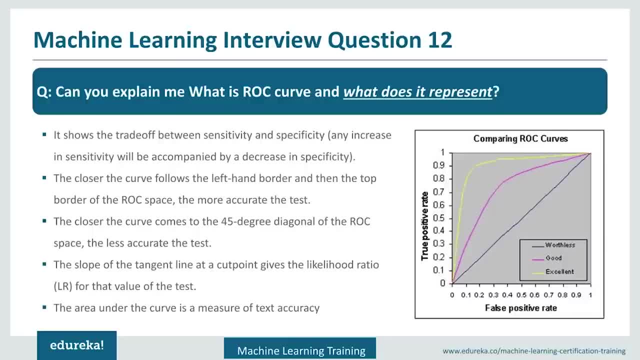 give some details about it and you can give the technical details, like how you can interpret it. First of all, it is like trade-off. There is always a trade-off between sensitivity and specificity, And one will increase in one will create a decrease in another. 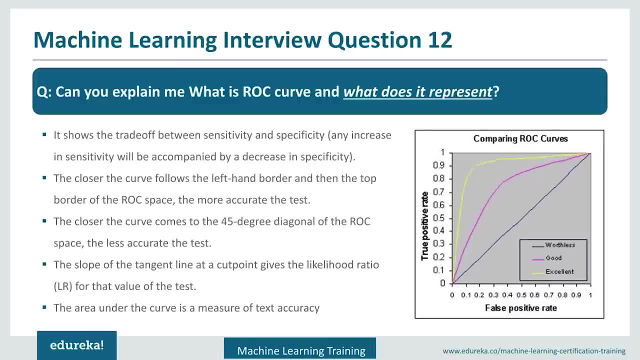 So it is really important. with the ROC curve you will see these differences as how they are getting impacted. The closer the curve follows to the true positive rate line and the more area it covers, such as the yellow one, as it is covering the highest area, that is more better than the pink one. 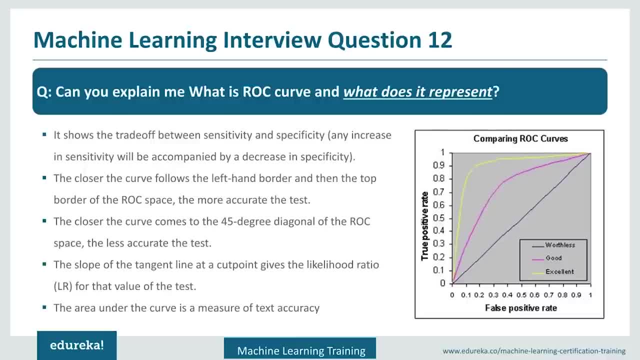 And pink one is more better than the blue one. The blue one is, as we already said, is like just a random guessing, with a 50% of probability, And the slope of the tangent line at the cut points gives you the likelihood ratio as how likelihood your model is. 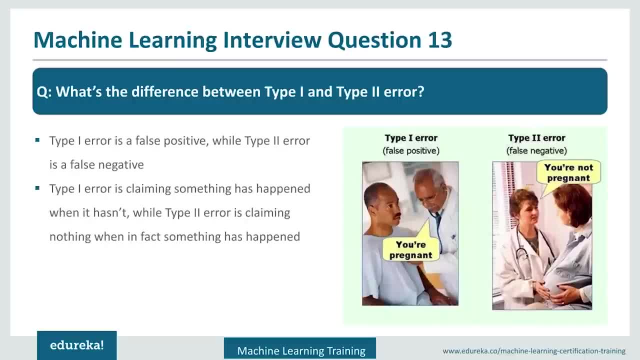 What's the difference between type 1 and type 2 error? So this is one of the very important concepts Which you interviewers trying to understand, as how you try to distinguish between the type of errors, Or do you understand, as how this type 1 and type 2 errors are impacting the performance of your model. 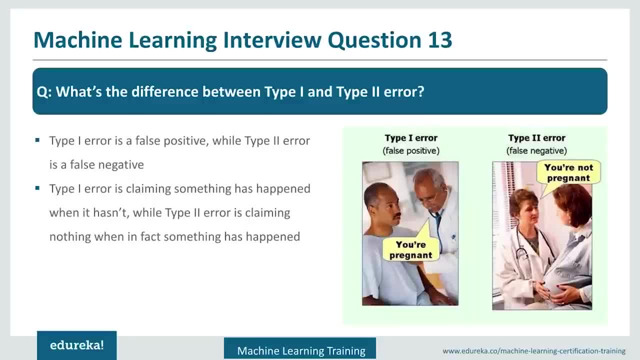 So interviewers trying to understand those things So you can give some good examples to say how these are going to impact. So first thing is type 1 error is false positives. So when something is not true which in actuality is not true, but your model is saying: 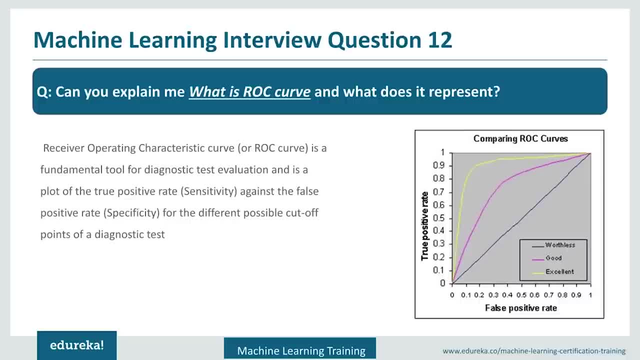 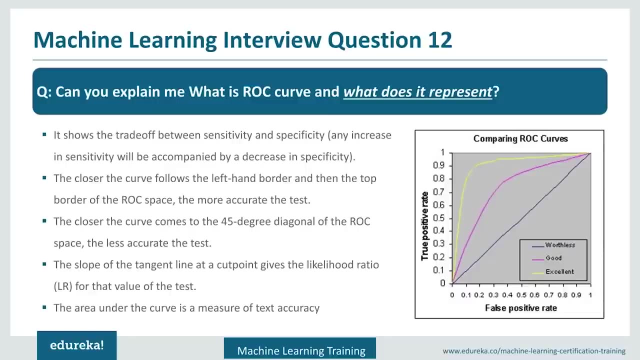 the better is the algorithm, so better you're trying to predict the true positive rates than the false negative rates. your true positive rates should increase faster than the false positive rates in this case. so first we saw like what actually ROC curve does, and we will see like 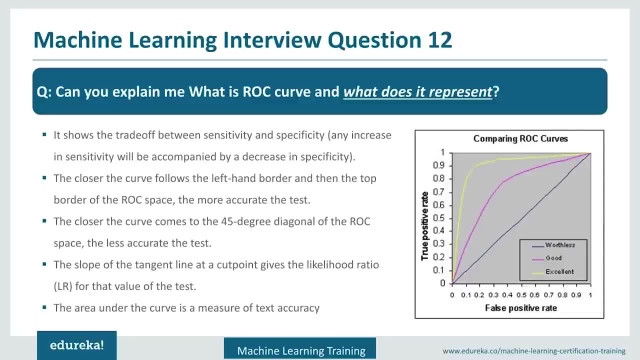 how you can interpret it now, so you can give the interviewer some idea about what is really ROC curve, give some details about it and you can give the technical details like how you can interpret it. so first of all, you can give the technical details like how you can interpret it. so first of 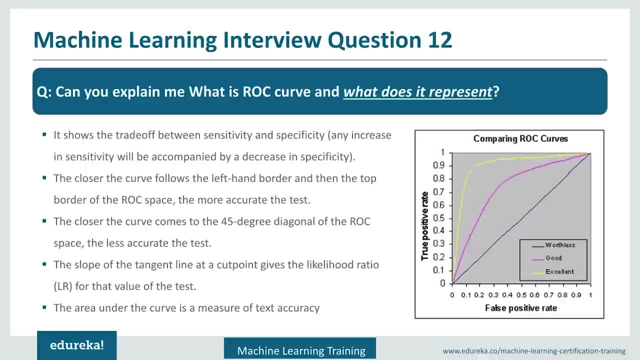 all you can give the technical details like how you can interpret it. so, first of all, it is like trade off. there is always a trade off between sensitivity and specificity and one will increase in one will create a decrease in another. so it is really important with the ROC. 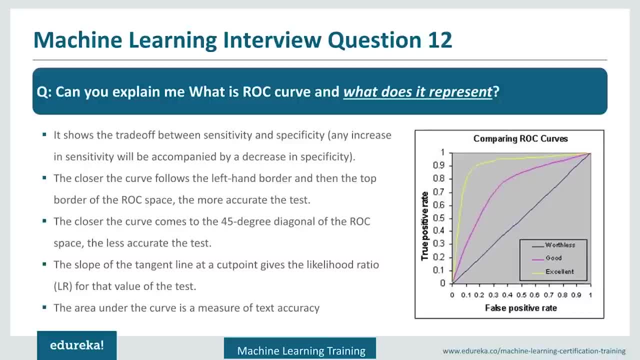 curve, you will see these differences as how they are getting impacted. the closer the curve follows to the true positive rate line and the more area it covers, such as the yellow one, as it is covering the highest area, that is more better than the yellow one. so they 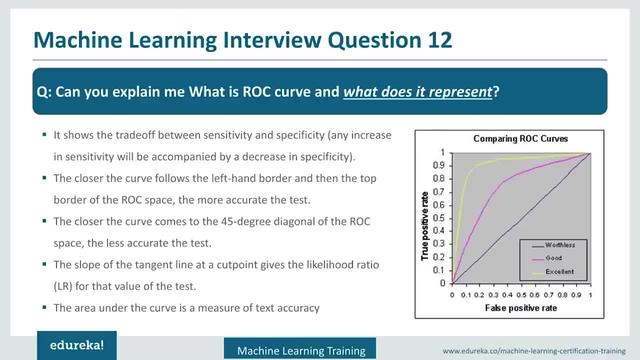 the pink one, and pink one is more better than the blue one. the blue one is, as we already said, is like just a random guessing, with a 50 of probability, and the slope of the tangent line at the cut points gives you the likelihood ratio, as how likelihood your model is. what's the? 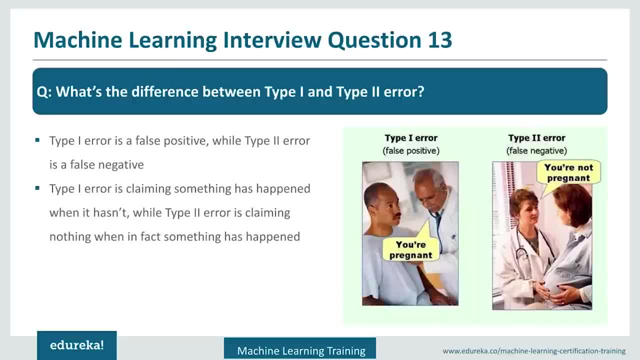 difference between type 1 and type 2 error. so this is one of the very important concepts which you interviewers trying to understand, as how you try to distinguish between the type of error. so do you understand, as how this type 1 and type 2 errors are impacting the performance of your model? 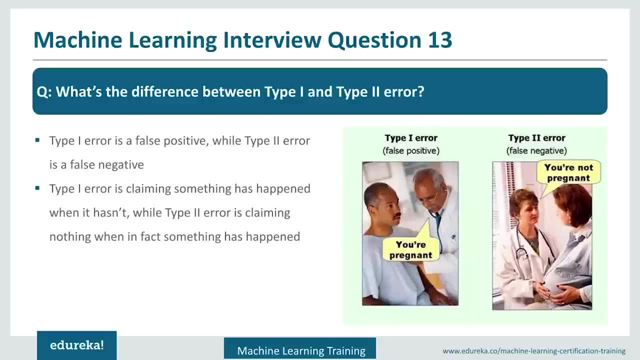 so interviews trying to understand those things so you can give some good examples to say how these are going to impact. so first thing is type 1 error is false positives. so when something is not true which in actuality is not true, but your model is saying it is true. 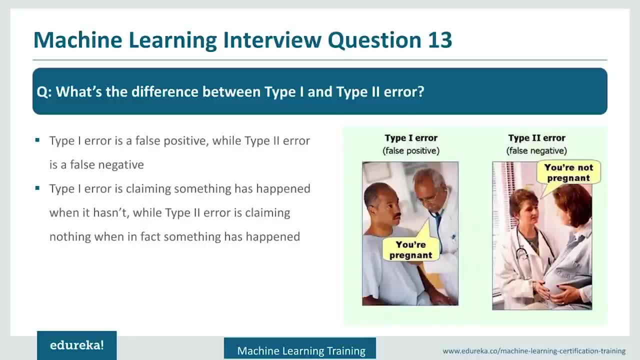 so, as we have the example, if a doctor says to a male person that he's pregnant, so it is like something is not true but you are saying it as true. so which is the false positive? and it's an example for the type one error, and the type two is a false negative. so when something 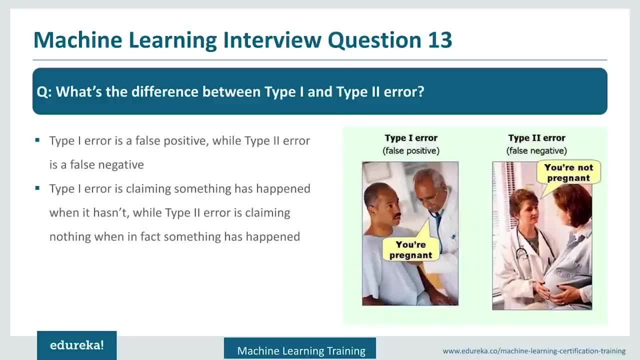 it is true. So, as we have the example if a doctor says to a male person that he is pregnant, So it is like something is not true, but you are saying it is true. So which is the false positive? and it's an example for the type 1 error. 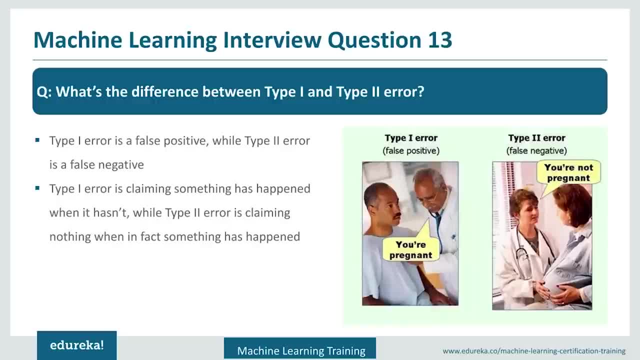 And the type 2 is a false negative. So when something you are saying is not there but in actuality is there. So when you're saying negative, so you are saying it is not there but in actuality it is false. 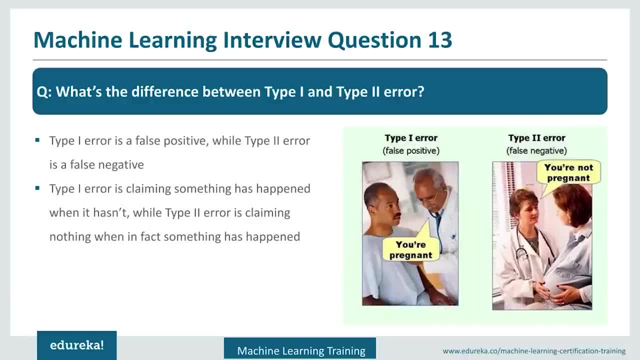 So that is the false positive. Similar example comes to where female is pregnant and the doctor says she is not pregnant. So this is like your model says something is not true, which is in the negative case, but in reality it is there. 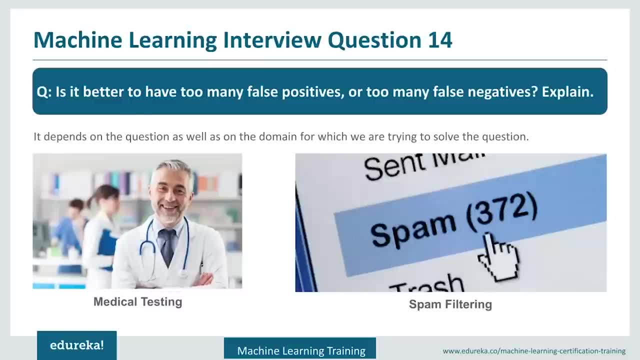 Is it better to have too many false positives or too many false negatives? This case really depends on the domain and the type of problem that you are solving. So, based on the different problems and the different Business requirements, you have to decide on what to have. 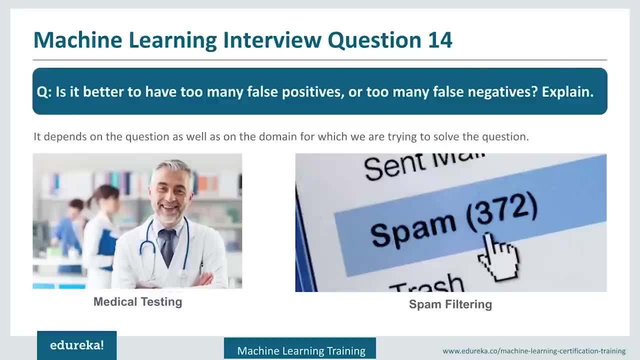 So there is always a trade off. You have to maintain the trade off between this false positive and false negatives and you have to decide which one we can keep as a more- As we already saw in the previous case, where you can imagine that, where a doctor sees a male person, that he is a pregnant person- 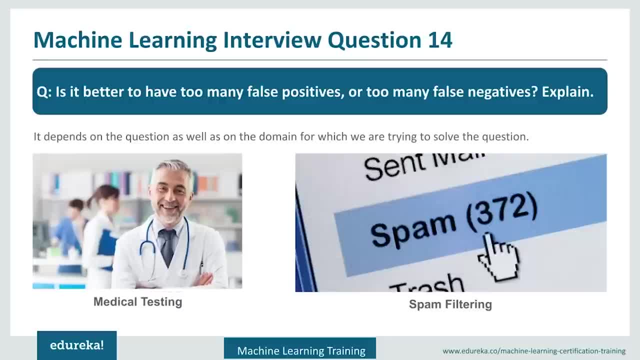 So these kind of model is always going to be a problem and you have to decide, like, how many of these cases you can manage. So is it like out of 100? Can you say that you can manage 10? Or how many you can consider for those, and you can move on with the model. 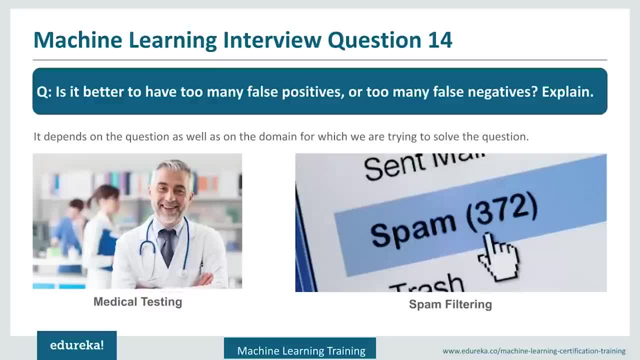 So similarly there is an example where in the spam filtering Can you say a good mail as a spam or not, So that trade-off you have to manage and based on that it will go. So this you have to define beforehand which one you can go on with. 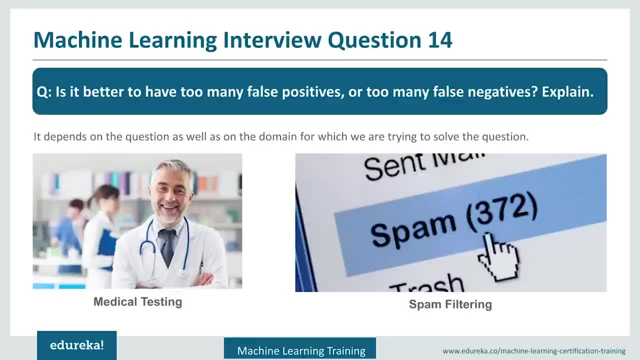 And you have to create a model as per that. So these kinds of questions are mostly related with the domain specific questions. So you can go ahead and base them in the domain specific questions questions, so you cannot just select any one of it and just give example. so 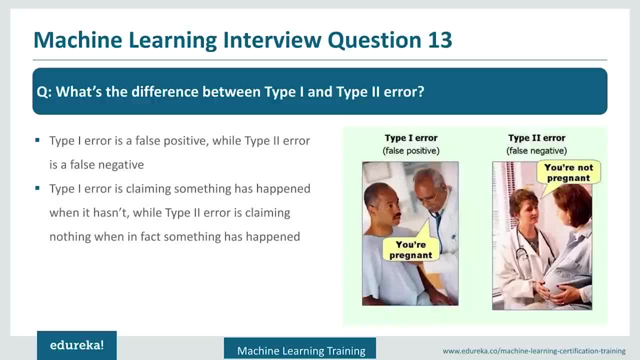 you are saying is not there, but in actuality is there. so when you are saying negative, so you are saying it is not that, but in actuality it is false. so that is the similar example comes to where female is pregnant and the doctor says she is not pregnant. so this 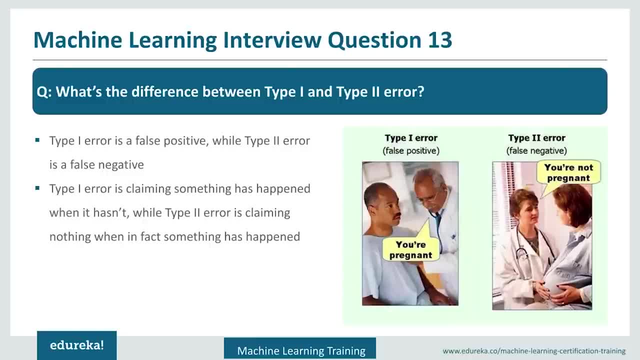 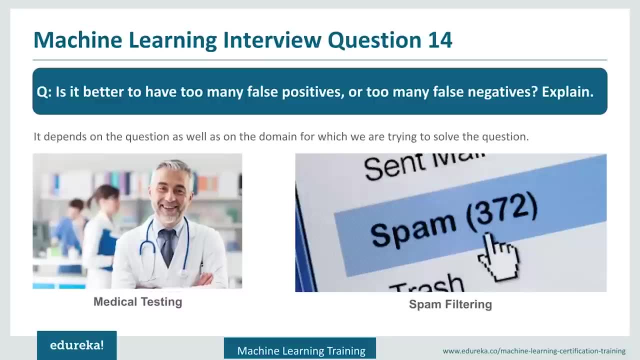 is like your model says something is not true, which is in the negative case, but in reality it is there. is it better to have too many false positives or too many false negatives? this case really depends on the domain and the type of problem that you are solving. so, based on the 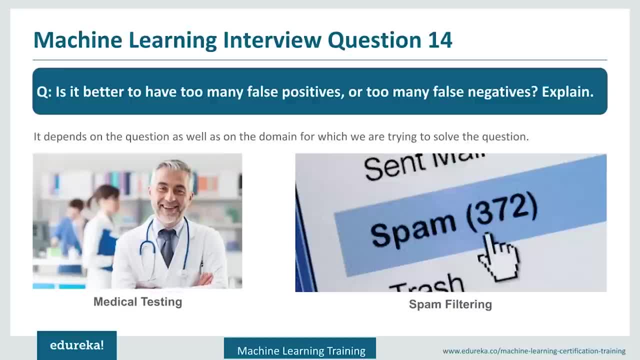 different problems and the different business requirements. you have to decide on what to have. so there is always a trade-off. you have to maintain the trade-off between this false positive and false negatives and you have to decide which one we can keep as a more, as we already saw in the previous case where you can imagine that, where a doctor says a male person. 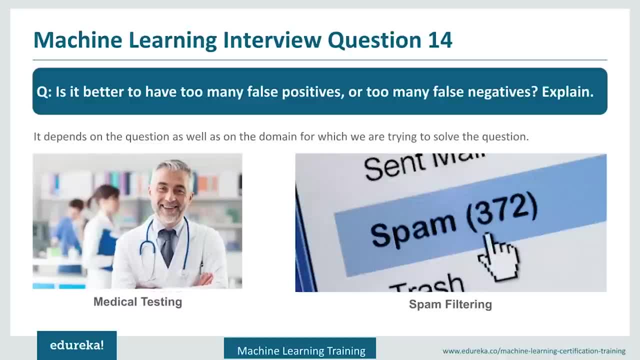 that he is an pregnant person. so this kind of model is always going to be a problem and you have to decide, like: how many of these cases you can manage? so is it like out of hundreds of cases you can manage? how many of these cases you can manage? so is it like out of? 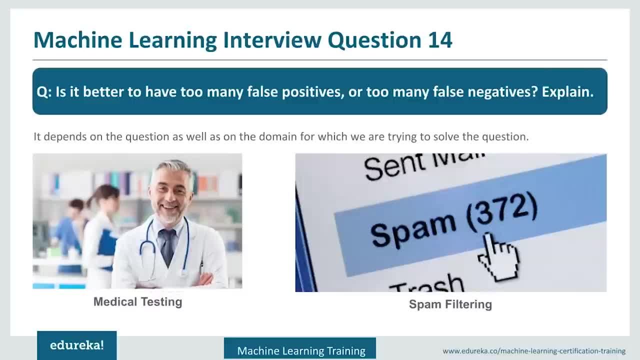 100, can you say that you can manage 10 false positives or how many you can consider for those, and you can move on with the model. so similarly, there is example where in this spam filtering so can you say a good male as a spam or not, so that trade-off you have to manage. 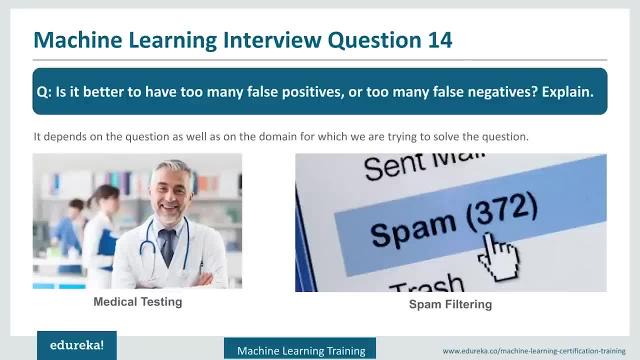 and based on that it will go. so this: you have to define beforehand which one you can go on with and you have to create a model as per that. so these kind of questions are mostly related with the domain, specific questions, so you cannot just select any one of. 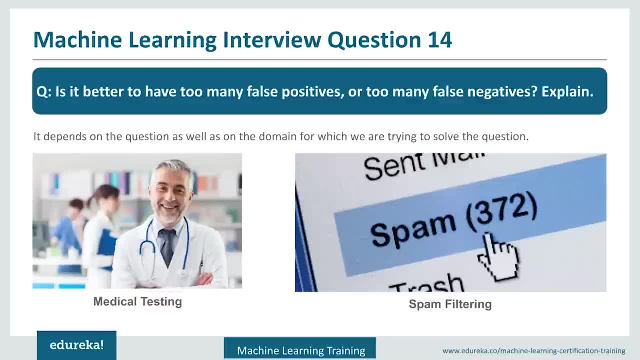 it and just give examples. so beforehand just try to understand what domain you are trying to explain and before that try to first be clear with what is false positives and what is false negatives. after that select a specific domains and give the examples. so, for example, in the medical testing, 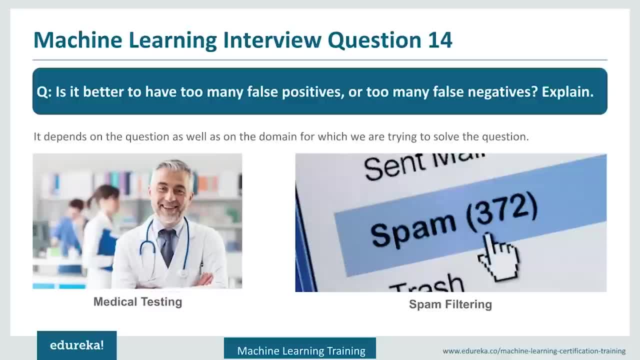 negatives may provide a false reassuring messages to the patients and physicians that some disease is absent. but you actually have to keep the false positives and positives in mind so you can give examples to give examples. so what will happen in this case is you are trying to give inadequate. 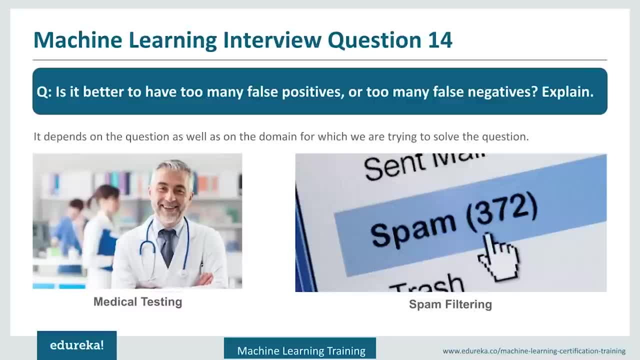 beforehand. just try to understand what domain you are trying to explain and before that try to first be clear with what is false positives and what is false negatives. after that select of specific domains and give the examples. so, for example, in the medical testing, negatives may provide a false reassuring. 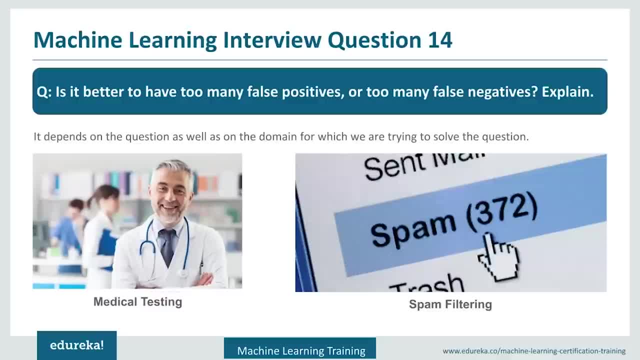 messages to the patients and physicians that some disease is absent, but you're actually saying it is present. so what will happen in this case is you are trying to give inadequate treatments to both the patients and the disease, which is not required, and these things will cost patients to the medical and the 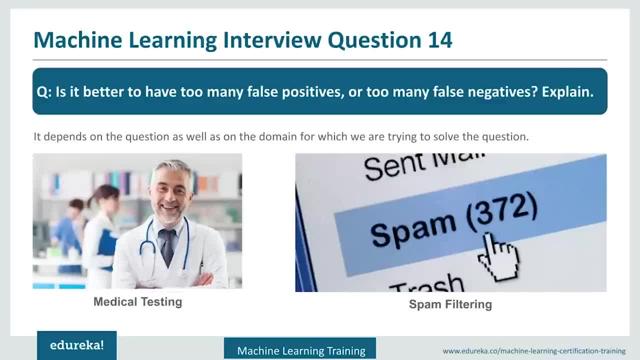 medical agencies and these kind of things has to be managed, so it is desirable to have many false positives in this case. the other example could be the spam filtering. so in this case a false positive occurs when spam filtering is blocking or wrongly classifying the legitimate emails. so you can't have that as many times, so users will get. 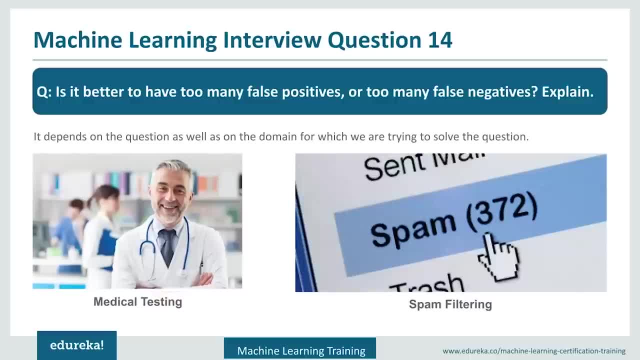 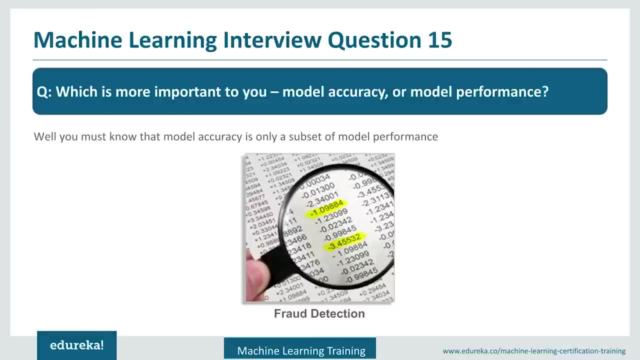 irritated when your actual mails are getting into the spam. so in this case, we prefer to many false negatives over the many false positives. so, based on the domain, it differs and you have to give the example specific to those domains. okay, so which is more important to you, the model accuracy or the model? 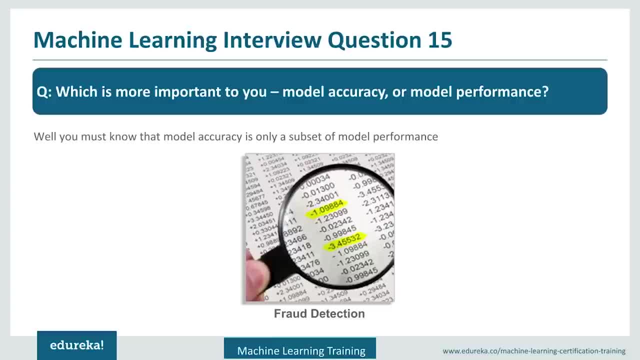 performance. this question they introduced trying to understand how better you know this terms. so do you really know the differences between this term? so first thing, try to understand what this terms are in. actually, the model accuracy is part of model performance. it is subset of the model performance. there are different model performance measures and model 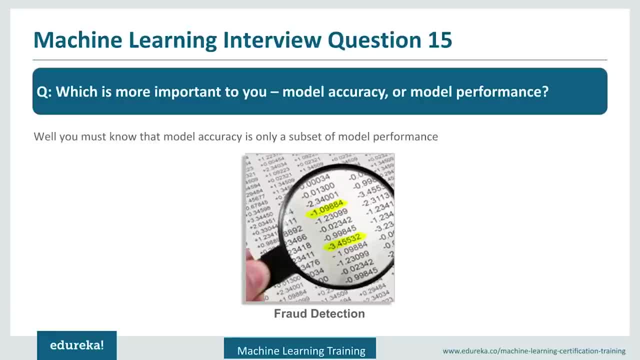 accuracy is one of them. so, for example, let's consider the case of fraud detection. so in this case, what will happen is you will have millions of rows and within those, only very less percentage of rows will have actual frauds. so in those cases, if you look for the model accuracy, your model accuracy. 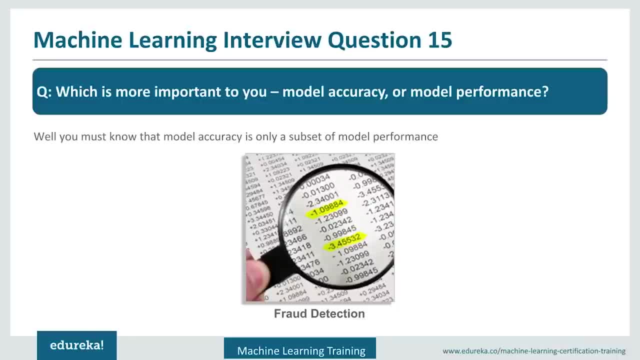 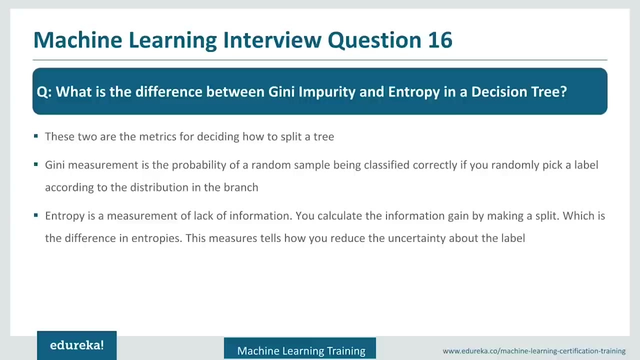 will mostly be higher and it won't give you a complete picture of your model performance. so model accuracy is just a subset of the model performance and there are more metrics that you have to look to understand the model performance. next question is: what is the difference between Gini impurity and entropy in? 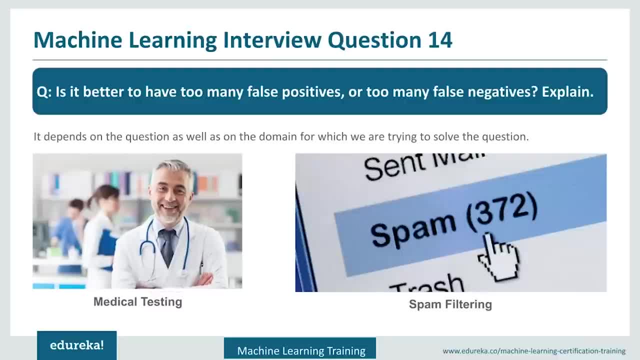 treatments to both the patients and the disease, which is not required, and these things will cost patients, to the medical and the medical agencies and these kind of things has to be managed. so it is desirable to have many false positives in this case. the other example could be the spam filtering. 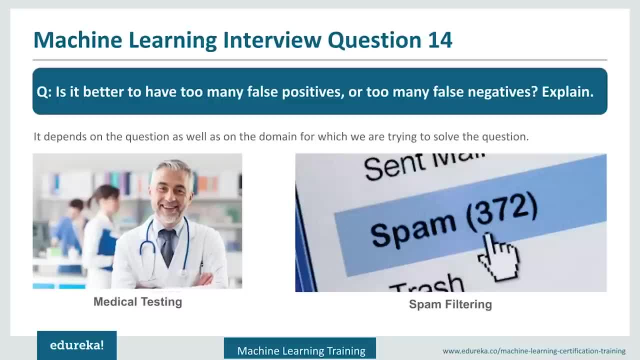 so in this case a false positive occurs when spam filtering is blocking or wrongly classifying the legitimate emails. so you can't have that as many times. so users will get irritated when your actual meals are getting into the spam. so in this case we prefer to many false negatives over the many. 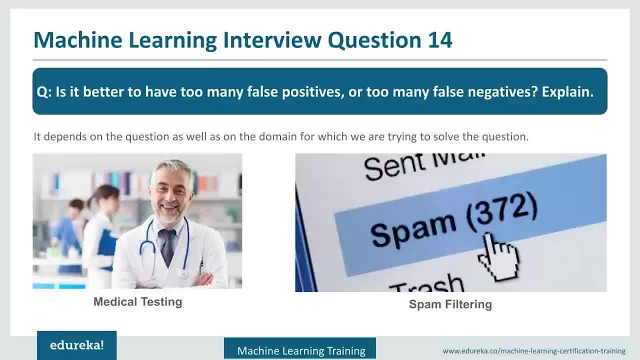 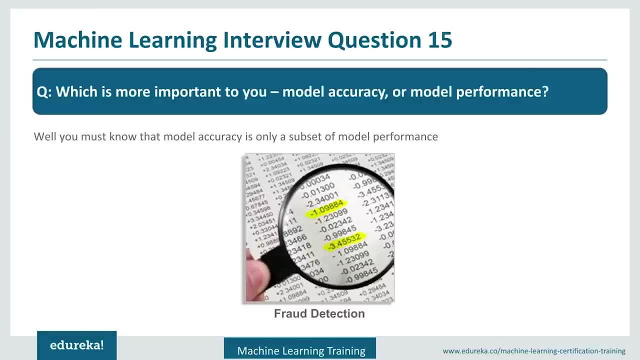 false positives. so based on the domain it differs and you have to give the example specific to those domains. okay, so which is more important to you, the model accuracy or the model performance? this question, the interview, is trying to understand how better you know these terms. so do you really know the differences between these terms? so, first thing, try to understand. 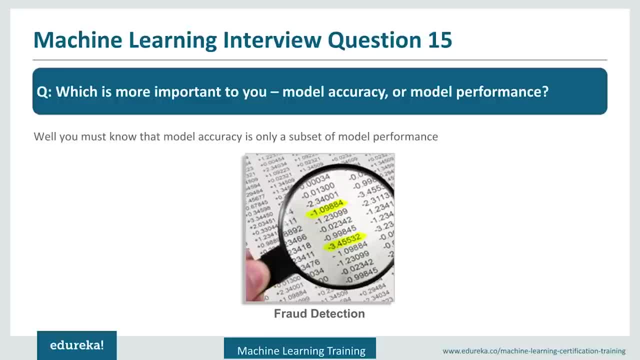 what these terms are in. actually, the model accuracy is part of model performance. it is subset of the model performance. there are different model performance measures and model accuracy is one of them. so, for example, let's consider the case of fraud detection. so in this case, what will happen is you will have millions of rows and within those, only very less. 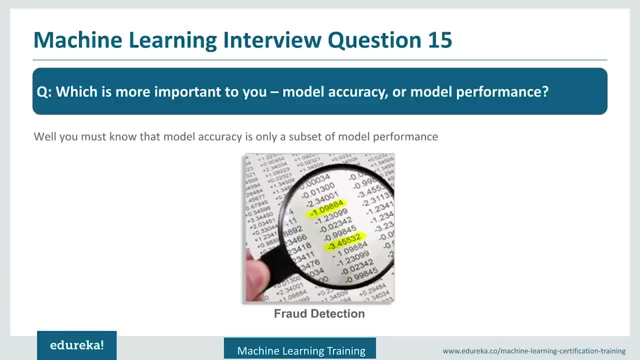 percentage of rows will have actual frauds. so in those cases, if you look for the model accuracy, your model accuracy will mostly be higher and it won't give you a complete picture of your model performance. so model accuracy is just a subset of the model performance and there are more metrics. 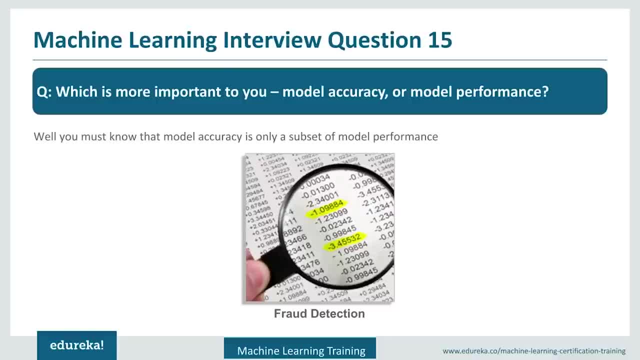 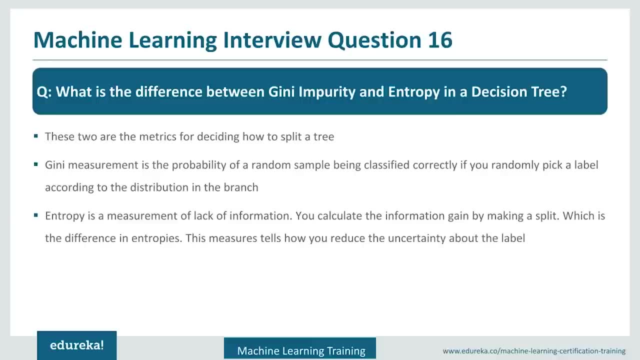 that you have to look to understand the model performance. next question is: what is the difference between the More Quality and Disclassified Monthly Plans, both things which are there? one of the reasons we would look at both. there's the problem with Mengers Leaf, and what we mean by that is they're not ready. we have a lot of simulations, then how do we? 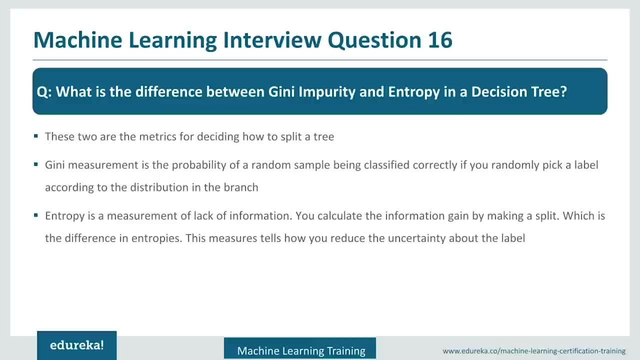 decision tree. so both first thing, this, both the things are used as a impurity measure in decision tree. what do we mean by impurity measure? so first you have to tell the interviewer what is really impurity in the decision tree. so impurity is something as how this classified your classes are within the tree, as when you. 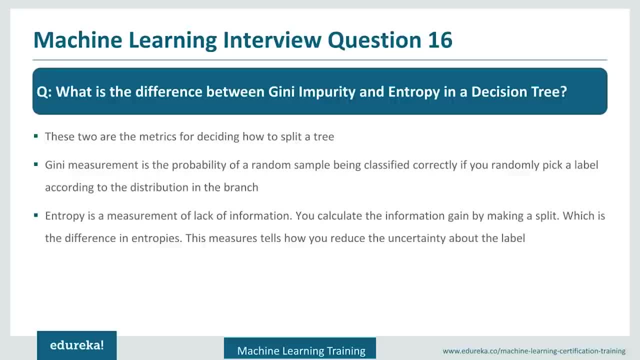 make a splits how your classes are getting split. so genie is one thing where what it does is it tries to see, as when you take a random sample out of the different labels, what is the chance of it's getting thick. it tries to add those probabilities and create an impurity. so it is basically one minus those. 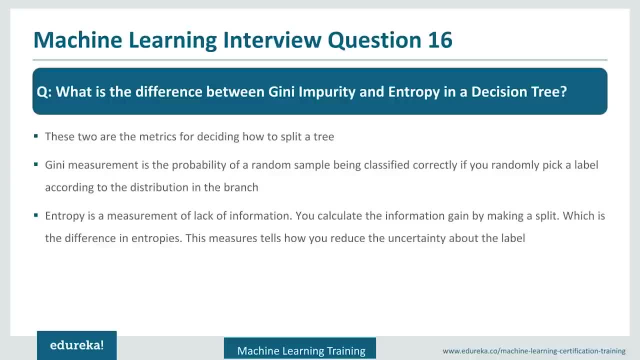 probabilities. the lesser it is, you're more confident that your labels are getting clustered in a different groups and different nodes. entropy is a measurement of lack of information, so when you are making a split within your data, it tries to identify as how this organized. this data is basically both. 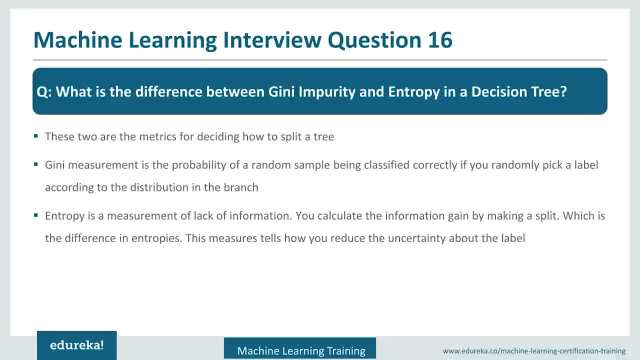 that trying to do a similar thing, but they are just doing it in a different manner with different mathematics. what happens is performance wise they both are same, but mostly people would go with genie, as it is less computationally overheading, as entropy uses a log function within the calculations, and that is bit. 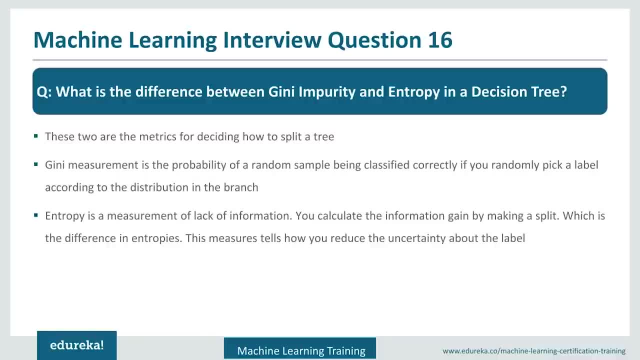 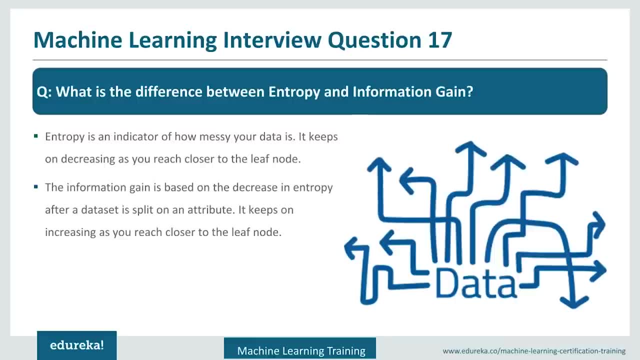 computationally expensive, so using genie it can be reduced, so mostly people would go with the genie. so what is difference between entropy and information gain? so when we are trying to make a split between genie and entropy, what happens when to make a split within the data? entropy is an indicator like how messy. 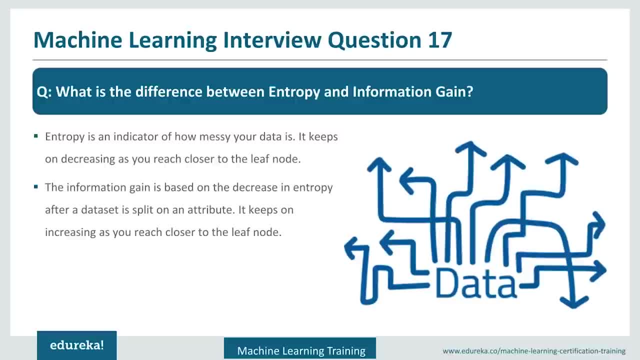 is your data within the nodes which you have. so as you keep on splitting the data based on the different features, you have the nodes and within those you have the labels, and entropy is giving you the major as how dis classified those are within your nodes. information gain is something which says how better you are. 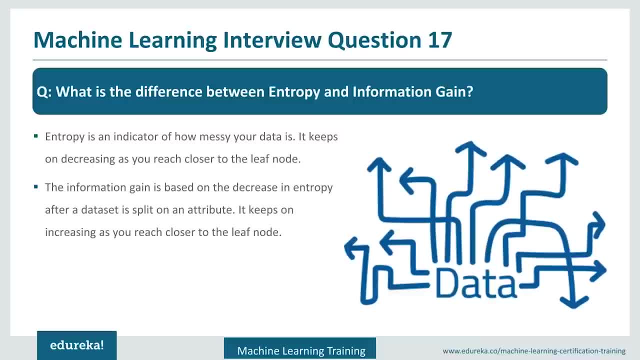 achieving the goal of separating your labels into different nodes. so you are. So as your entropy keeps on decreasing, your information gain keeps on increasing. So both are related with each other, and as your entropy is decreasing, your information gain will keep on increasing. 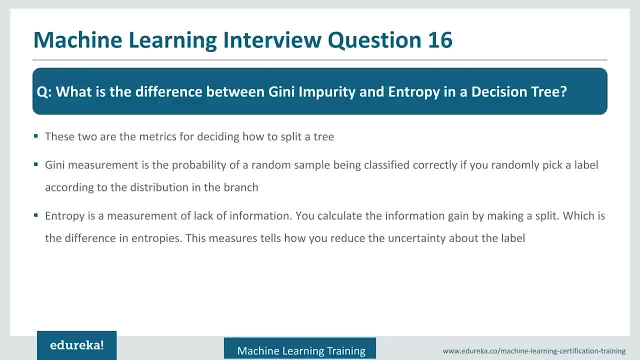 analyze as you compare them. what use graphs do gridscom stuff to a ganska. it goes like sample out of the different labels. what is the chance of it getting thick? It tries to add those probabilities and create an impurity. So it is basically one minus those probabilities. 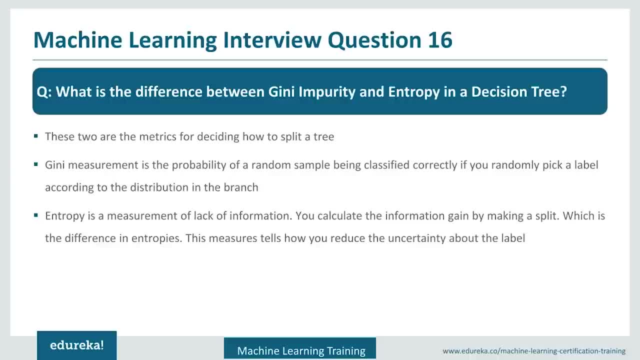 The lesser it is, you're more confident that your labels are getting clustered in different groups and different nodes. Entropy is a measurement of lack of information, So when you're making a split within your data, it tries to identify as how disorganized this data is. 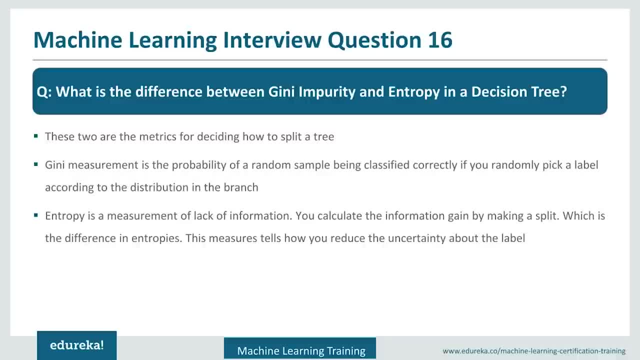 Basically, both are trying to do a similar thing, but they are just doing it in a different manner with different mathematics. What happens is, performance-wise, they both are same, but mostly people would go with Gini as it is less computationally overheading, as 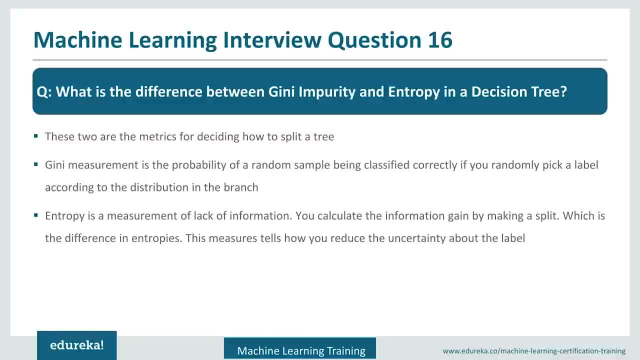 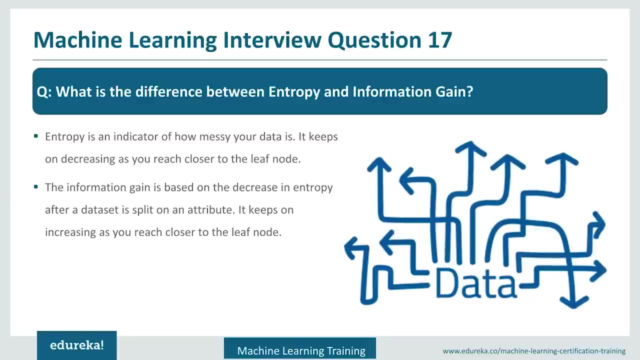 entropy uses a log function within the calculations and that is bit computationally expensive. So using Gini it can be reduced, so mostly people would go with the Gini. So what is the difference between entropy and information gain? So when we're trying to make a split within the data, 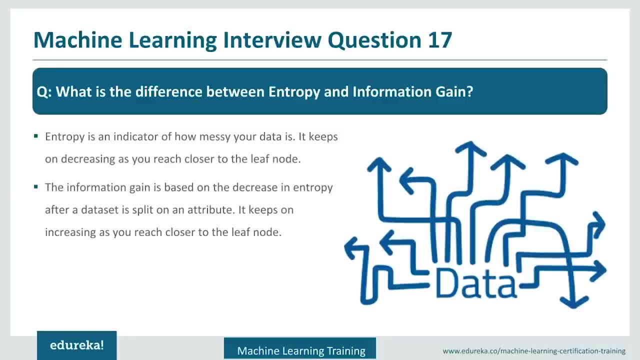 entropy is an indicator like how messy is your data within the nodes which you have. So, as you keep on splitting the data based on the different features, you have the nodes and within those you have the labels, and entropy is giving you the measure as how disclassified those are within your nodes. 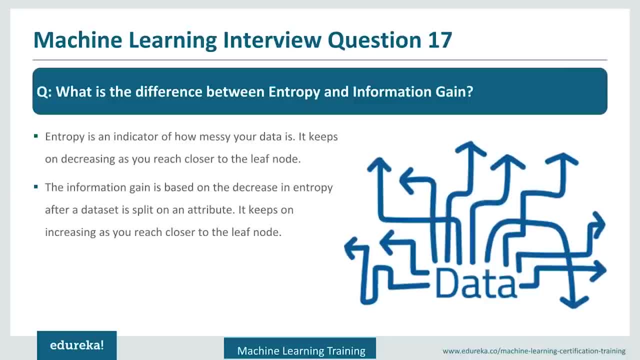 Information gain is something which says how better you are achieving the goal of separating your labels into different nodes. So as your entropy keeps on decreasing, your information gain keeps on increasing. So both are related with each other and as your entropy is decreasing, your information gain will keep on increasing. 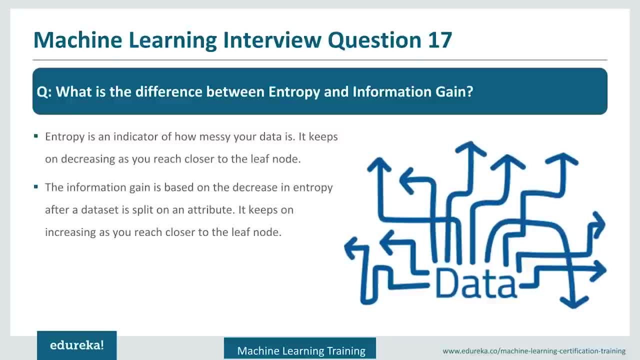 Your information gain will keep on increasing as your nodes are getting pure and pure. So Node purity basically says, as you're getting specific classes within the nodes, those nodes are getting purer. So when we are trying to take specific classes, like our classes are getting segregated based on the tree and the 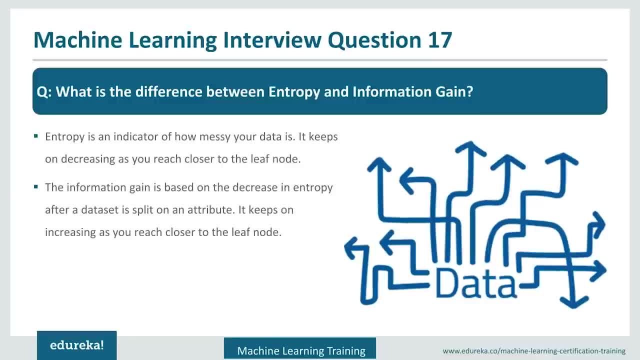 nodes are getting purer and purer, So information gain will keep on increasing as we are moving toward the leaf nodes, and the nodes are getting purer and our entropy will keep on decreasing as we are reaching closer to the leaf nodes. What is overfitting and how do you ensure you are not? 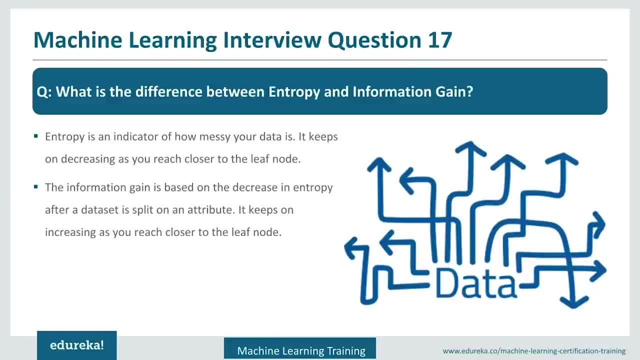 Your information gain will keep on increasing as your nodes are getting pure and pure. So node purity basically says, as you are getting specific classes within the nodes, those nodes are getting purer. So when we are trying to take specific classes, like our classes are getting segregated based on the tree and the nodes are getting purer and purer. 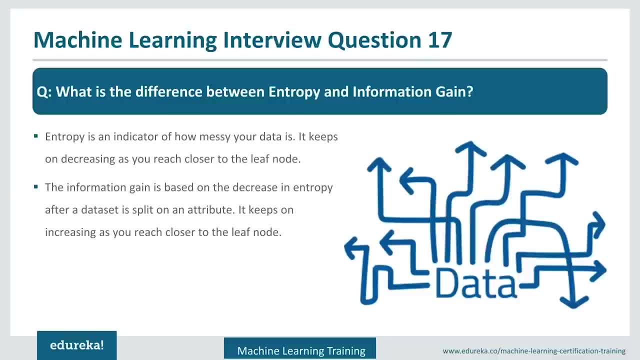 So information gain will keep on increasing as we are moving toward the leaf nodes, and the nodes are getting purer and our entropy will keep on decreasing as we are reaching closer to the leaf nodes. What is overfitting and how do you ensure you are not overfitting with a model? 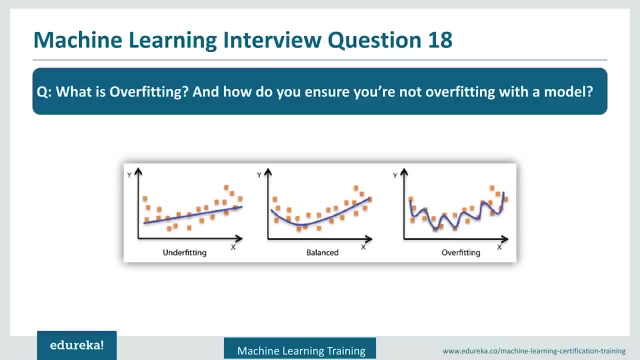 So overfitting is really important concept within the modeling performance And your interviewer is really interested to understand as how you are confident with those terms and how you can explain those So that once you explore those things, interviewer is interested to see, as you know, the machine learning models in the right terms or not. 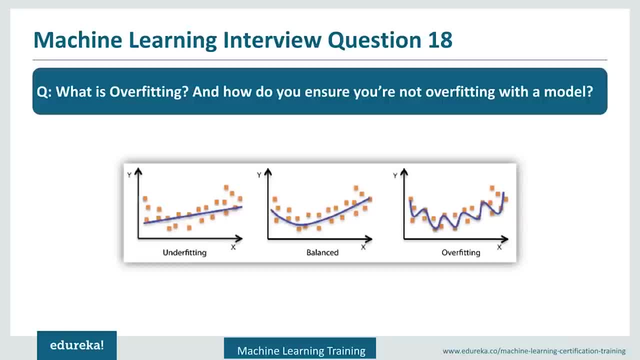 So once you prove the fitting of your model, there could be three different ways that your model is getting fitted. So first is the case of underfitting. In underfitting, what is happening is your model is not learning completely what is there within the data. 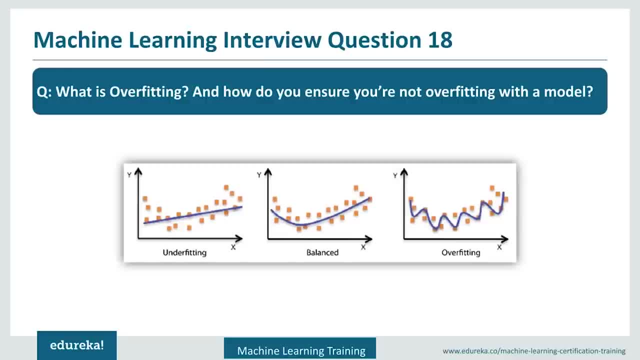 It is bypassing, It is biased to a specific set of data and it is not learning the patterns which are there within the data. So when new data comes in, it won't be able to classify it properly or regress it properly. Balanced is a balanced condition where what's happening is your model is learning the patterns within the data in a very generalized manner. 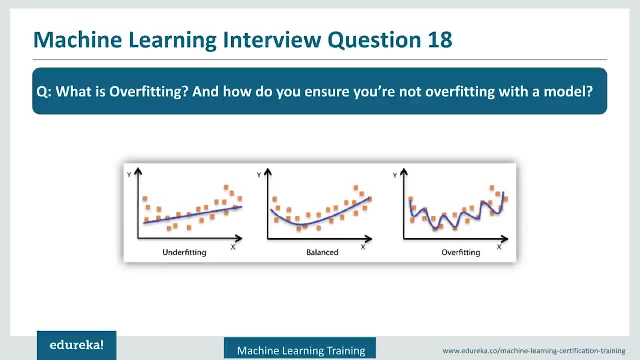 What do you mean by generalized is your model is learning it on the training data. plus, when you give it a new testing data, it is still able to generalize it what was there in the training data. Overfitting is something which is like very much closely getting fitted with the data which is there within the training set. 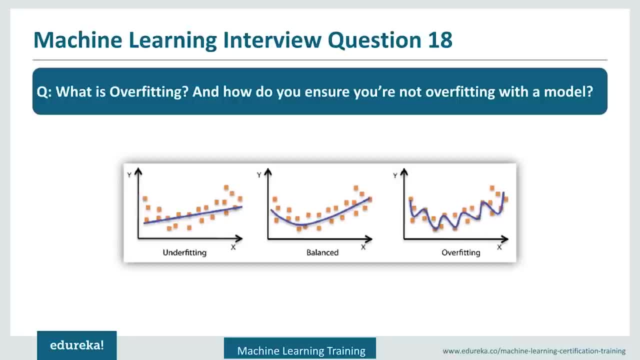 So it is getting very much closer. It's creating a curve, as you see in the diagram, very much closer to the data which is there within the training. So when you give it a new testing data, it won't generalize it very well. 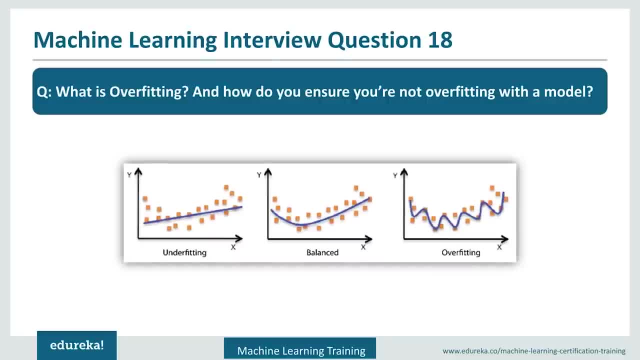 So you have to be sure, in overfitting, it's trying to create a model which is very much learning all the parameters in an exact manner from the training data, Which shouldn't be the case. The next part is: how do we ensure our model is not overfitting? 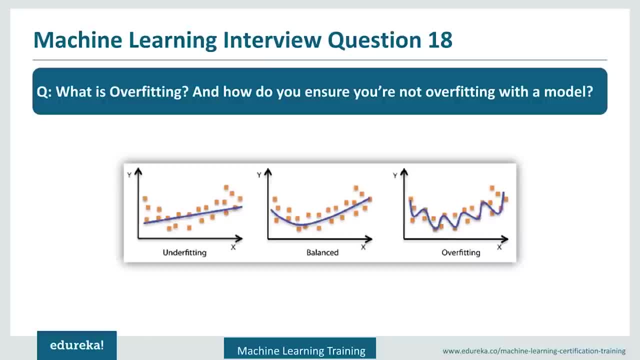 overfitting with the model. So overfitting is really important concept within the modeling performance and your interviewer is really interested to understand as how you are confident with those terms and how you can explain those So that once you explore those things, interviewer is interested to see, as you know, the machine learning models in the right terms or not. So 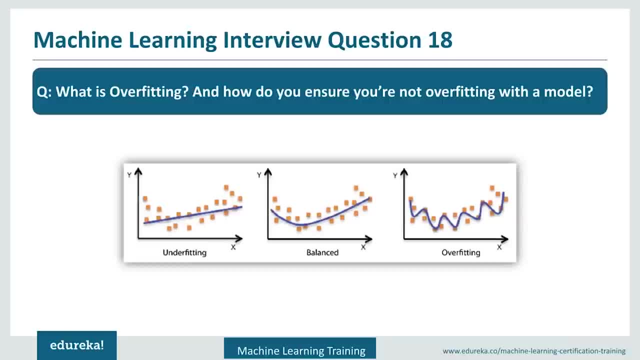 once you prove the fitting of your model. there could be three different ways that your model is getting fitted. So first is the case of underfitting. In underfitting, what is happening is your model is not learning completely what is there within the data. 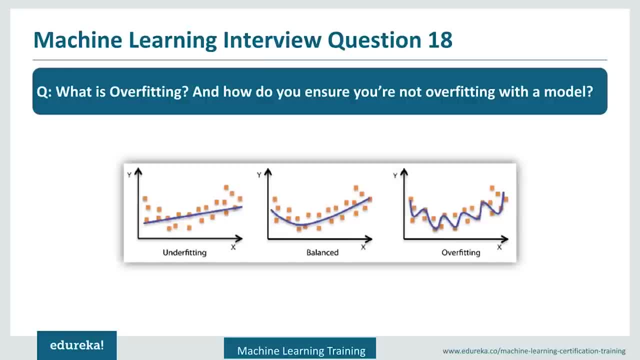 It is biased to a specific set of data and it is not learning the patterns which are there within the data. So when new data comes in, it won't be able to classify it properly or regress it properly. Balanced is a balanced condition where what is happening is your. 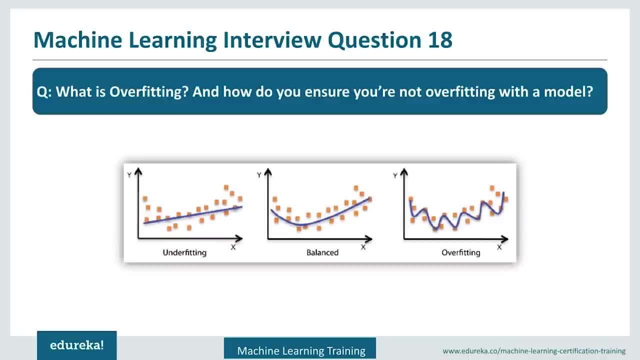 model is learning the patterns within the data in a very generalized manner. What do you mean by generalized is your model is learning it on the training data. plus, when you give it a new testing data, it is still able to generalize it. what was there in the 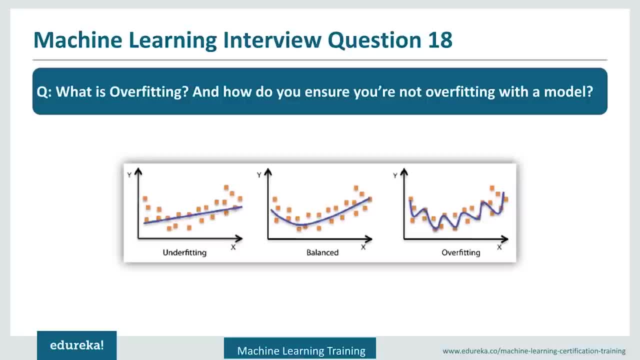 training. data Overfitting is something which is like very much closely getting fitted with the data which is there within the training set. So it is getting very much closer. it's creating a curve, as you see in the diagram, very much closer to the data which is there within the training. 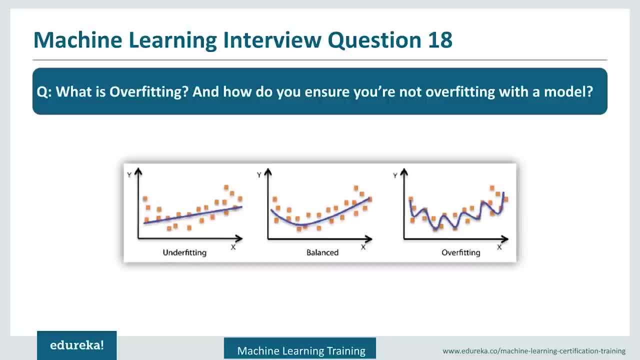 So when you give it a new testing data, it won't generalize it very well. So you have to be sure, in overfitting it's trying to create a model which is very much learning all the parameters in an exact manner from the training set. So that's the first thing that you need to do. 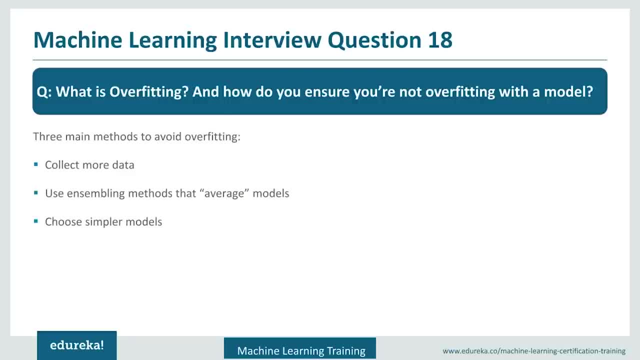 The next part is: how do we ensure our model is not overfitting? So for this there are multiple ways that we can control the overfitting. First is we collect more data. So as we have lesser data, our model will try to get very much exact to what is there within the training data: Getting more. 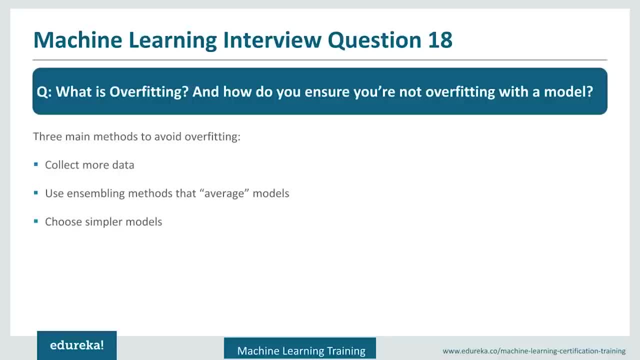 data may help it to generalize well. Second is using ensemble methods that average the models. So when we split our data into models, we get more data and we can control the overfitting. So this is how we use multiple components or we use multiple models, which will try to understand data in a 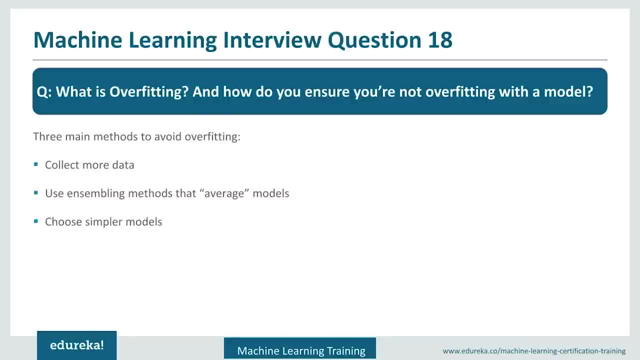 So for this there are multiple ways that we can control the overfitting First is we collect more data. So as we have lesser data, our model will try to get very much exact to what is there within the training data. 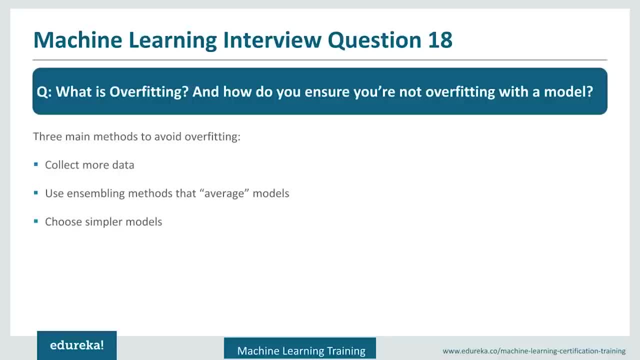 Getting more data may help it to generalize well. Second is using ensemble methods that average the models. So when we split our data into multiple components Or we use multiple models, which will try to understand data in a different manner, Each model within ensemble will try to understand the data in a different manner. 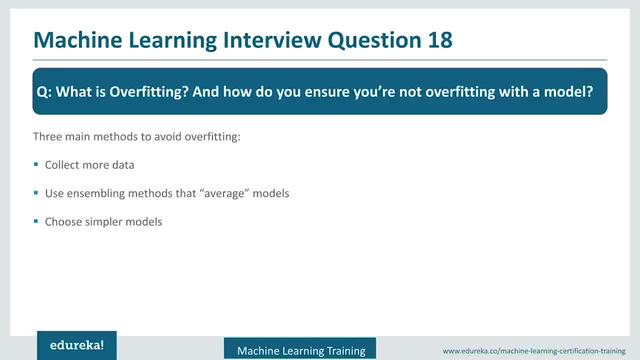 They'll try to capture the different patterns And when you try to average those, your overfitting will reduce a bit. Choosing, simpler models. So simpler models are like logistic regressions, where you understand what is happening. In logistic regression you will get a parameters as how the coefficients are there with each of your features. 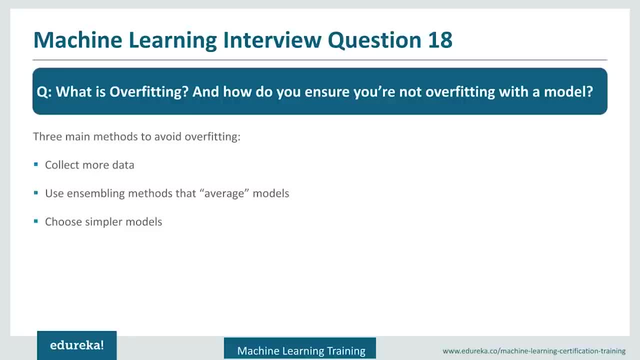 So you can try to understand what is really happening and try to make some tweaking to the model with the simpler models. Few more thing is you can try to add regularization. So there are regularizations called L1 and L2, which basically penalizes your model when it tries to overfit or underfit. 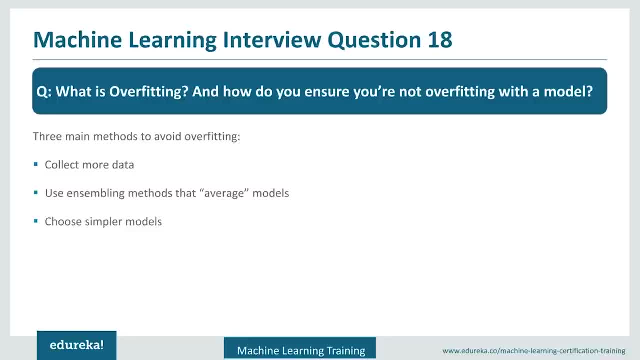 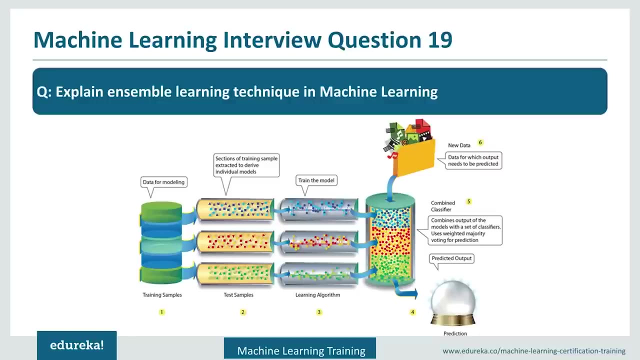 It tries to balance your data and it doesn't let it overfit or underfit. You can set the boundaries of how stricter you want to be with the regularization. That is the fourth step. Explain ensemble learning technique in machine learning. So first of all you have to explain. 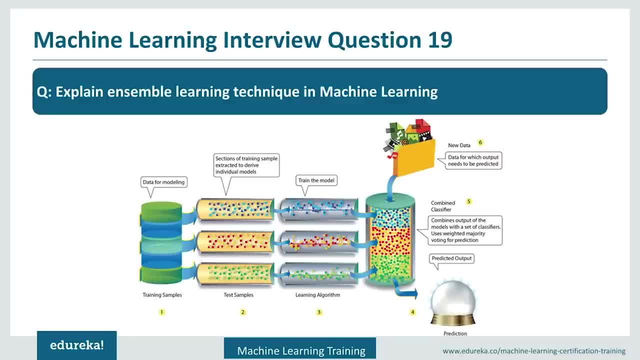 So interviewer is interested to see how you can explain the theoretical part of it plus the practical part of it. First, as a theory, ensemble is nothing but different models combined together and each model is trying to understand the data in a different manner. So each model will try to capture different patterns within the data. 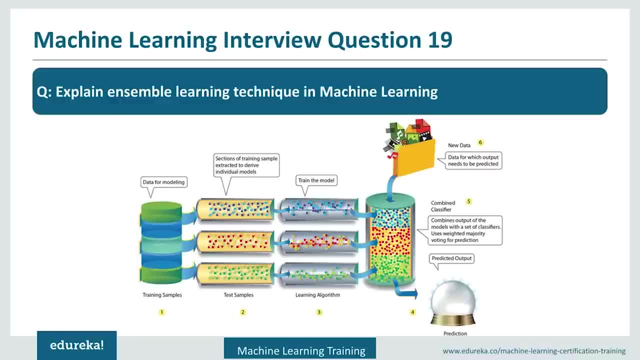 All are weak learners, So in this case they are called all are weak learners And when we combine them together, they become a better model. A single model is created out of it, which is a better predictor model. So if you see the example which is there below, it is like we are feeding this different set of data and we are creating different models. 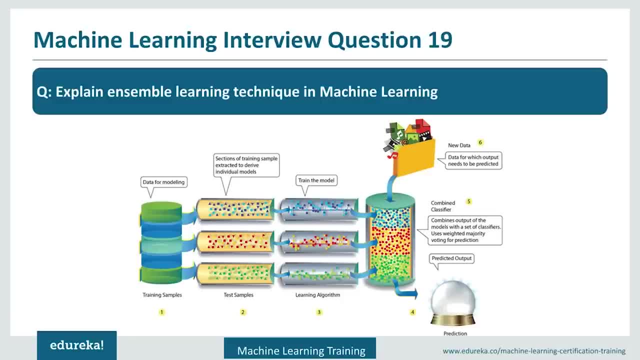 So these are the different models which are creating out of the different samples of our data and this- all models- are combined into a single model And, based on the new data, output of all these models are combined together and your single output is created by merging all the outputs of different models. 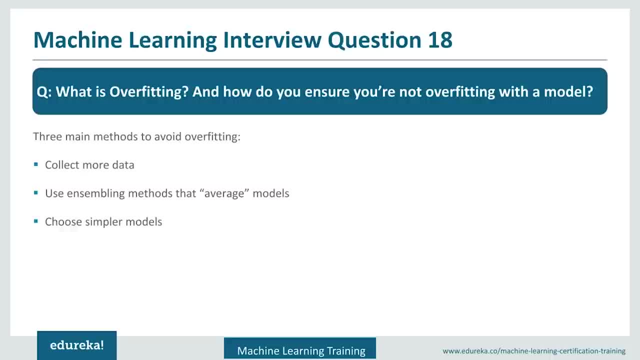 different manner. Each model within ensemble will try to understand the data in a different manner. They'll try to capture the different patterns and when you try to average those, your overfitting will reduce a bit Choosing simpler models. So simpler models are like logistic regressions, where you 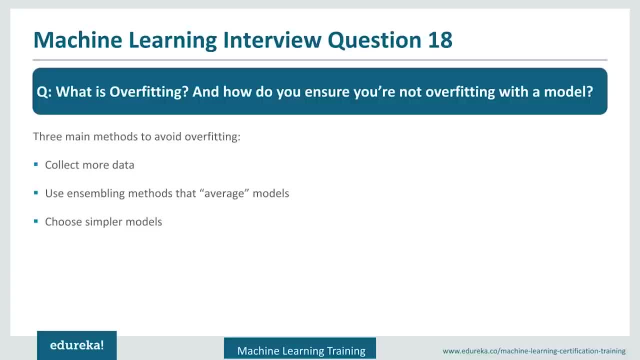 understand what is happening In logistic regression. you will get a parameters as how the coefficients are there with each of your features. So you can try to understand what is really happening and try to make some tweaking to the model with the simpler models. Few more thing is you can try to add regularization. So there are 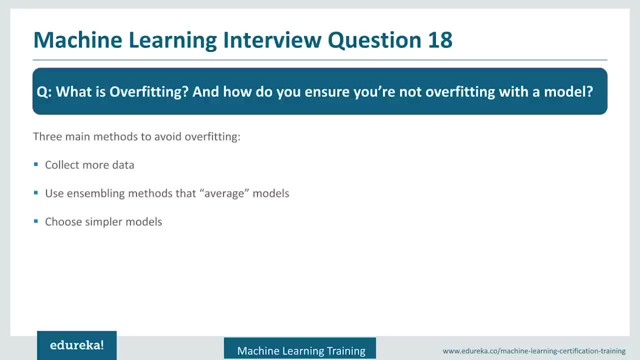 regularizations called L1 and L2, which basically penalizes your model when it tries to overfit or underfit. It tries to balance your data and it doesn't let it overfit or underfit. You can set the boundaries of how stricter you want to be with the regularization, So that's how you can try to. 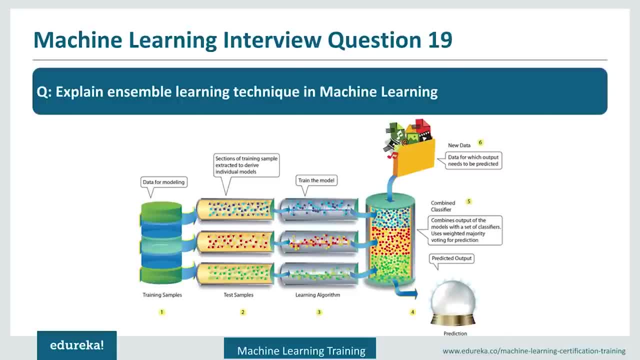 overfit your model. So that's the fourth step: Explain ensemble learning technique in machine learning. So first of all you have to explain. So interviewer is interested to see how you can explain the theoretical part of it plus the practical part of it First, as a theory, ensemble is nothing but. 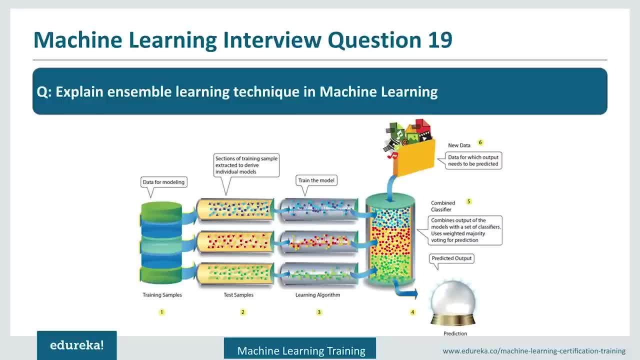 different models combined together and each model is trying to understand the data in a different manner, So each model will try to capture different patterns within the data. All are weak learners, So in this case they are called. all are weak learners and when we combine them together, they 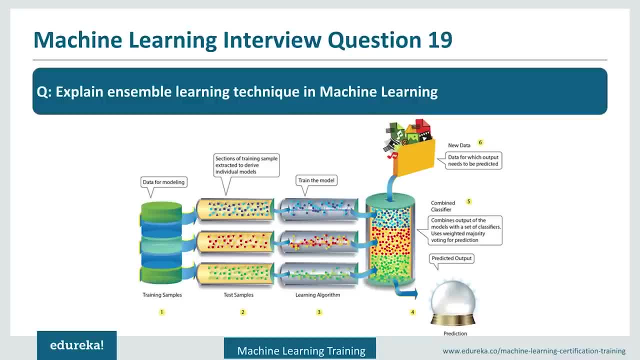 become a better model. A single model is created out of it which is a better predictor model. So if you see the example which is there below, it is like we are feeding this different set of data and we are creating different models. So these are the different models which are creating out of the 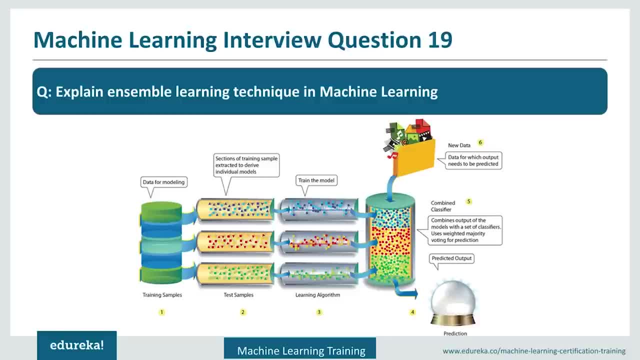 different samples of our data and this- all models- are combined into a single model and, based on the new data output of all these models are combined together and your single output is created by merging all the outputs of different models. So in the case of regression, it is mostly 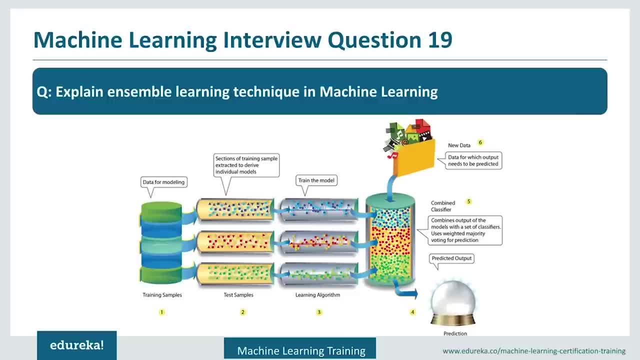 like. you try to average those values and create a new value. In the case of classification, you try to take the majority of all those. So ensemble learning is basically learning from committee or crowd. So you basically train a large number of models and then try to combine their predictions. 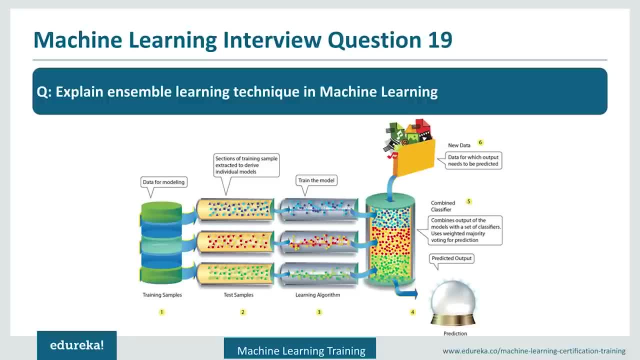 So in the case of regression, it is mostly like you try to average those values and create a new value. In the case of classification, you try to take the majority of all those. So ensemble learning is basically learning from committee or crowd. 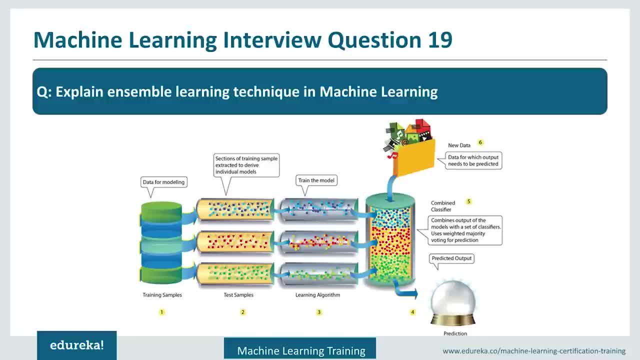 So you basically train a large number of models And then try to combine their predictions and create a single conclusion out of it. So, for example, when we split our data set into different samples and those, each sample is fed into a similar kind of algorithm, for example the decision tree. 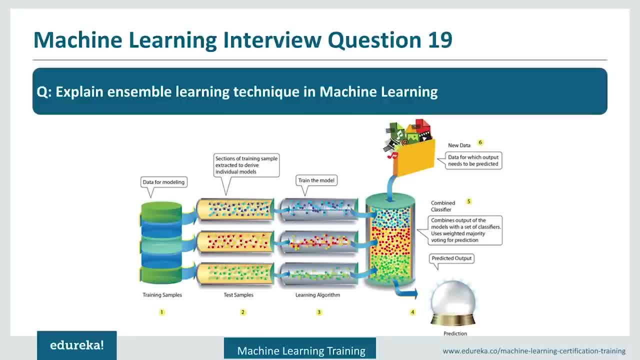 So we create 100 decision trees on 100 samples of our data and each model is trying to capture different patterns of your data. In the end, we try to average all the outputs of this hundred models and we take a single output, So the ensemble models power. 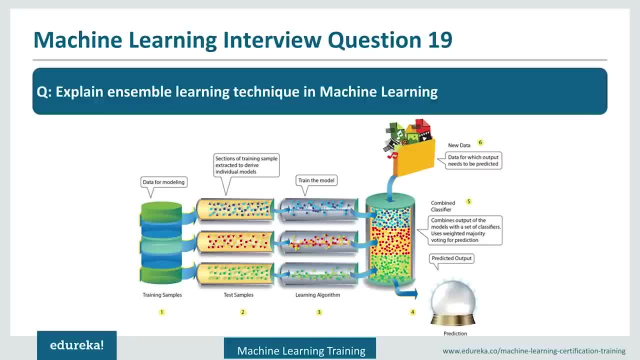 Power is very different and they are very popularly used to control the overfitting of your models. So there are two components. There are two types which are there in the ensemble model. One is the bagging and the other is the boosting. 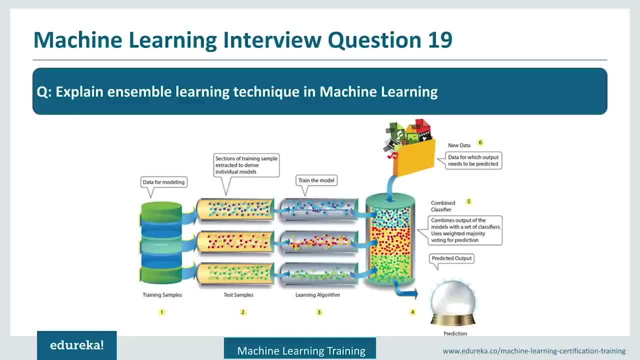 So you can just give the theory about, like, how both of them works. So boosting is something where what we are doing is we are trying to sample the data. Different samples are trained on similar kind of algorithms, such as the decision trees, the logistic regression or the SVM. 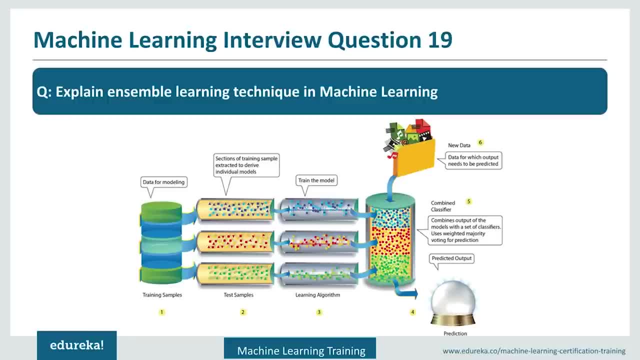 On all samples, a single algorithm is used and at the end you combine all the outputs of this models and that is the output of the bagging and boosting is the algorithm where what happens is your. each model is trying to understand the misclassification which are there within the previous model and try to learn those. 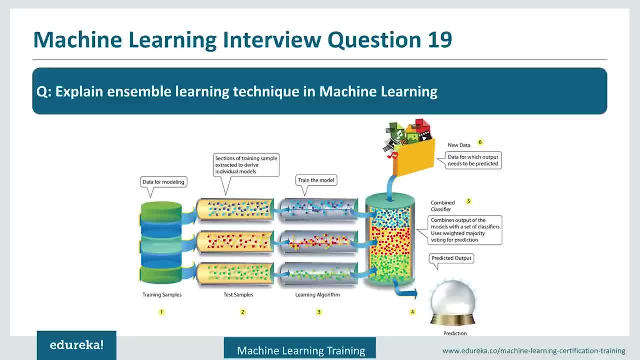 So each model, the next model, will try to learn the misclassification which are there within the previous model and become better and better, and again, The combined output of all this is taken to create a ensemble of it and use it. Yeah, So this example is similar to bagging algorithm, where what is happening is we have a different samples of data and we are using it. model: 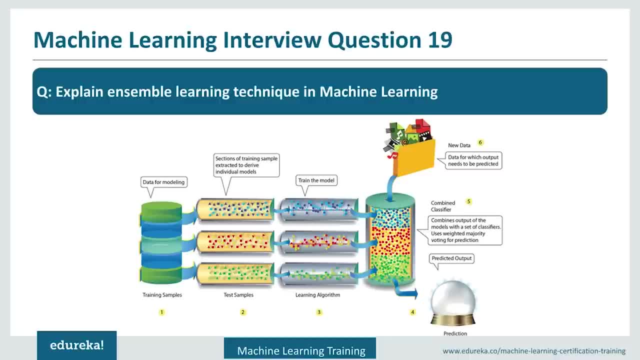 So let's assume we are using a decision tree in this case. So we are training decision trees on each of this models and, in the end, output of this models are being fed to a whole ensemble and ensemble model. It will try to aggregate all the decisions. 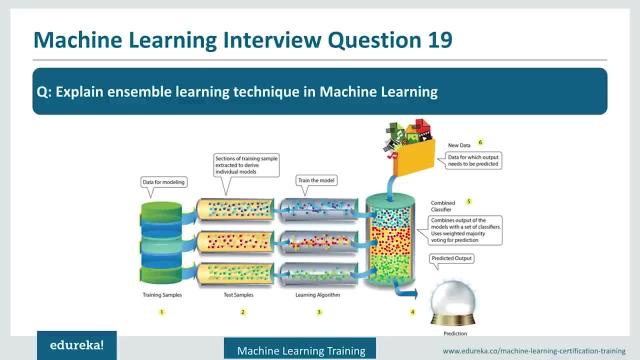 and create a single conclusion out of it. So, for example, when we split our data set into different samples and those, each sample is fed into a similar kind of algorithm, For example the decision tree. So we create 100 decision trees on 100 samples of our data and each model is trying to capture. 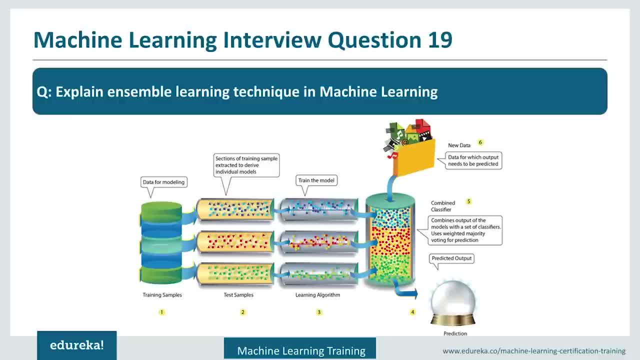 different patterns of your data. In the end we try to average all the outputs of these 100 models and we take a single output. So the ensemble model's power is very different and they are very used to control the overfitting of your models. So there are two components, there are two types. 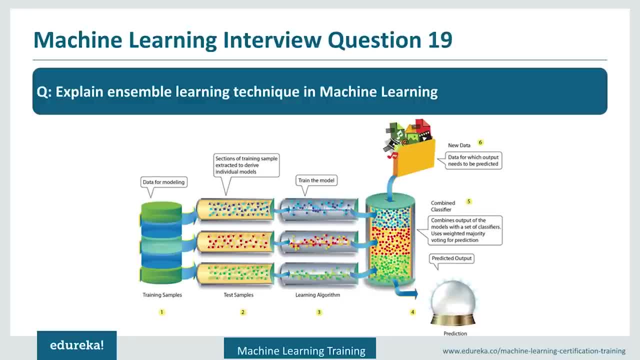 which are there in the ensemble model. One is the bagging and the other is the boosting, So you can just give the theory about like how both of them works. So boosting is something where what we are doing is we are trying to sample the data. Different samples are trained on similar kind of algorithms. 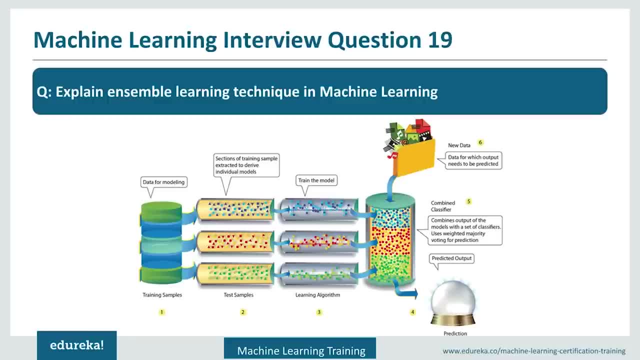 such as the decision trees, the logistic regression or the SVM. On all samples, a single algorithm is used And at the end you combine all the outputs of these models and that is the output of the bagging And boosting is the algorithm where what happens is your. each model is trying to understand the 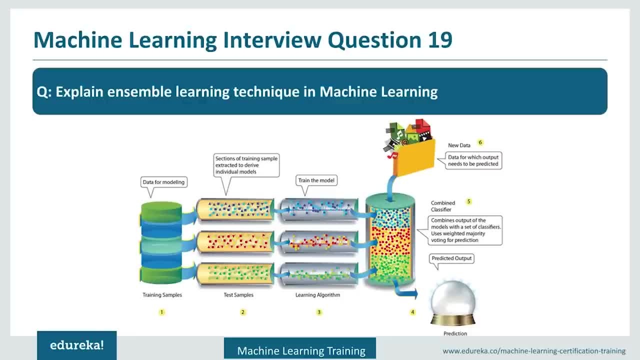 misclassifications which are there within the previous model and try to learn those. So each model, the next model will try to learn the misclassifications which are there within the previous model and become better and better And again the combined output of all this is taken to. 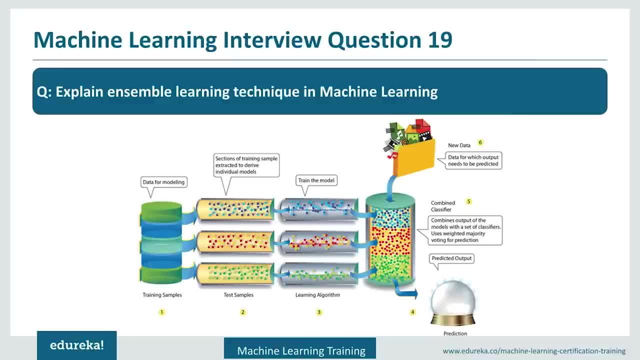 create a ensemble of models, So this example is similar to a bagging algorithm. that what is happening is we have a different samples of data and we are using the model. so let's assume we are using a decision tree in this case. So we are. 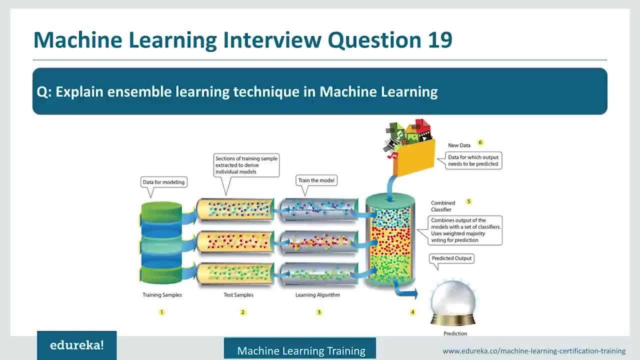 training decision trees on each of these models and, in the end, output of this models are being fed to a whole ensemble and ensemble model. it will try to aggregate all the responses from this models and give a single output. So, as a single learner can't do this whole together would do so. that is the 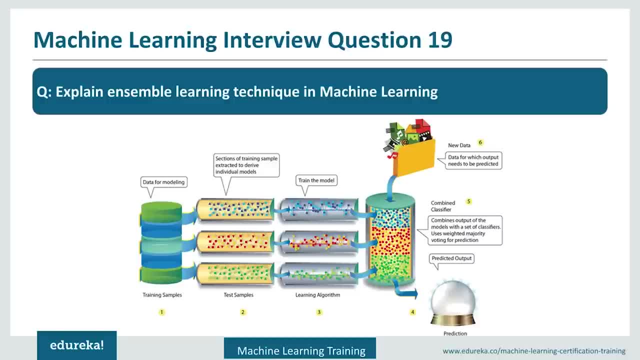 Responses from this models and give a single output. So, as a single learner can't do this whole, together would do so. that is the power of ensembles, as each one is trying to learn different parts of it and give you a single output which is more powerful than the single algorithm. 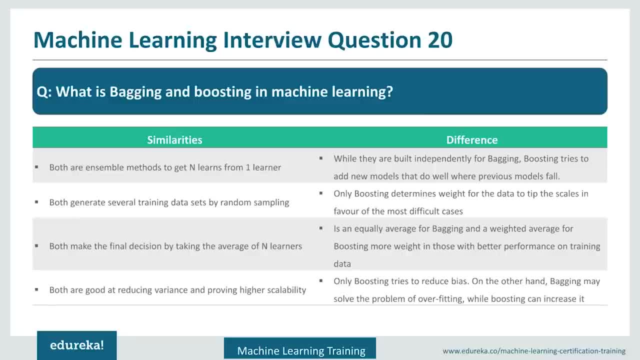 So what is bagging and boosting in machine learning? both bagging and boosting are nothing but the types within the ensemble models and, as we know, ensemble models are nothing but collection of different models. They're Also called as the weak learners, and we combine all these weak learners output to create a single learner, which is a better predictor of your than the all weak learners. 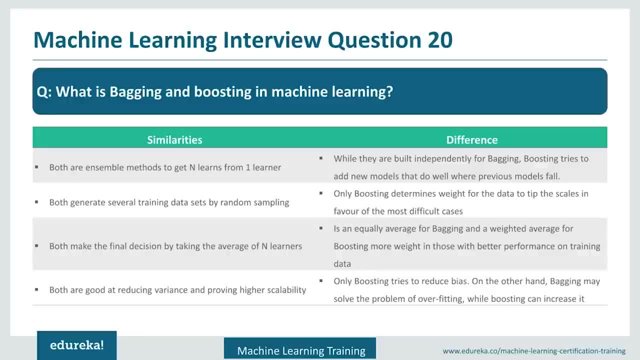 So both generate data from the sample. So you take a random sample sort of your data. It is mostly with the replacement, as you take a data and you again replace it and you again take a different sample of it. It's called the random sampling of your data. 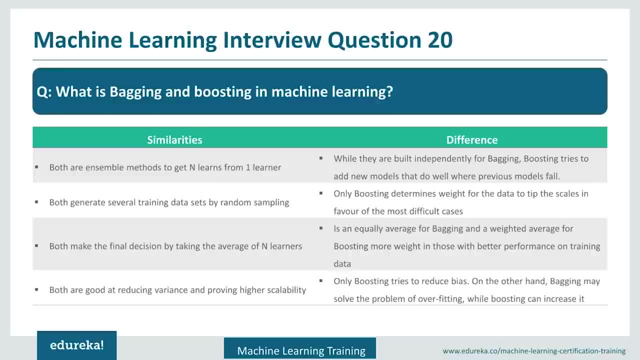 So in both the cases all the weak learners are Are aggregated to create the final output. So in the case of classification, you try to take the class which is coming as the highest. if you're training a hundred models and you have a binary classification, assume that out of hundred models, if 80 models are predicting that your class one should be there and 20 models are predicting your class two should be there, then in ensemble class one would be selected as output. in the case of regression, 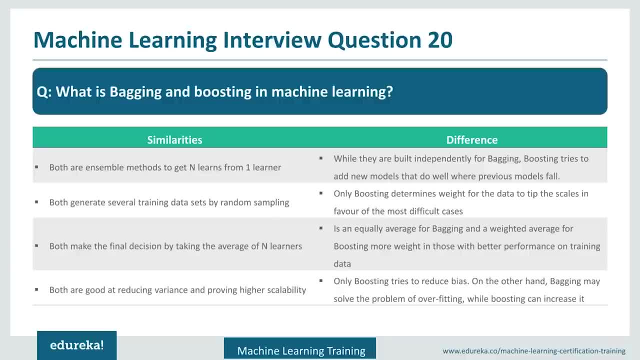 It is like you're trying to average all the outputs. As it's a continuous data, You try to aggregate all the output from the different models, So both are good at reducing the variance. So as both are good at reducing the variance as they are trying to learn different models. 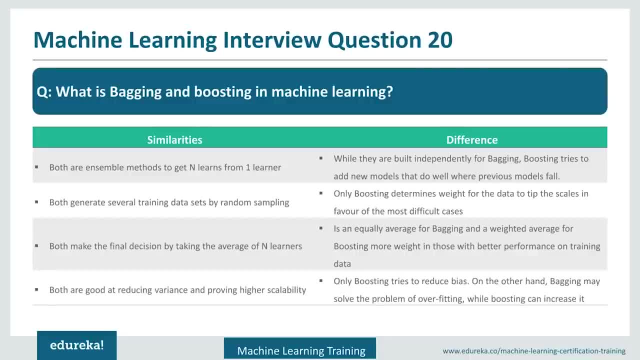 They reduce the overfitting of your data and, in effect, they also reduce the variance which is available within that model. So, as part of the differences, boosting what it does is it tries to learn different weak learners, is different. Samples are created and each sample is trained on a similar model. 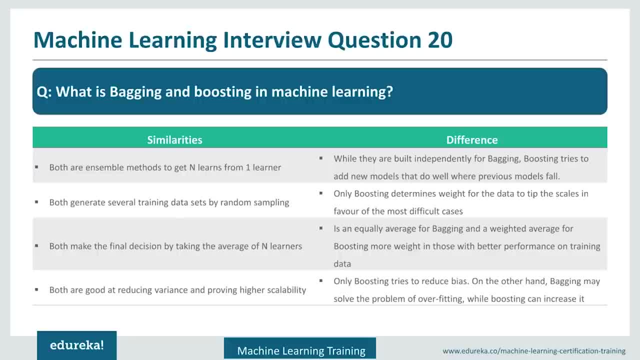 So, for example, if you are using decision tree, on all sample we use decision tree and each one predicts their performance, Whereas in boosting what it does is it tries to learn from the mistakes that the previous model has performed. each model is a better version of the previous model. 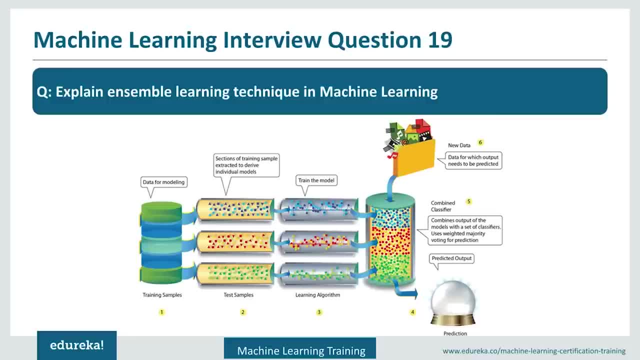 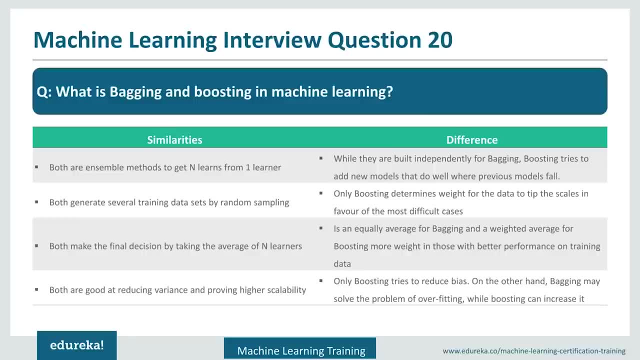 power of ensembles, as each one is trying to learn different parts of it and give you a single output which is more powerful than the single algorithm. So what is bagging and boosting in machine learning? Both bagging and boosting are nothing but the types within the ensemble models and, as we know, ensemble 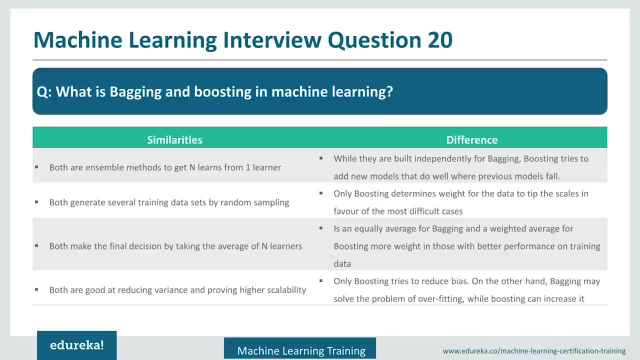 models are nothing but collection of different models. they are also called as the weak learners and we combine all these weak learners output to create a single learner which is a better predictor of your than the all weak learners. So both generate data from the sample, so you take a random sample sort. 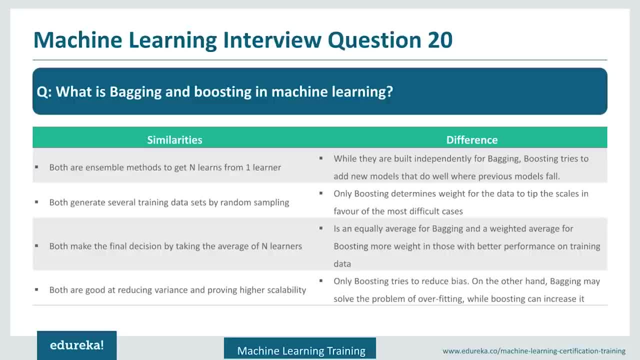 of your data. it is mostly with the replacement, as you take a data and you again replace it and you again take a different sample of it. It's called the random sampling of your data. So in both the cases, all the weak learners are aggregated to the single learner. 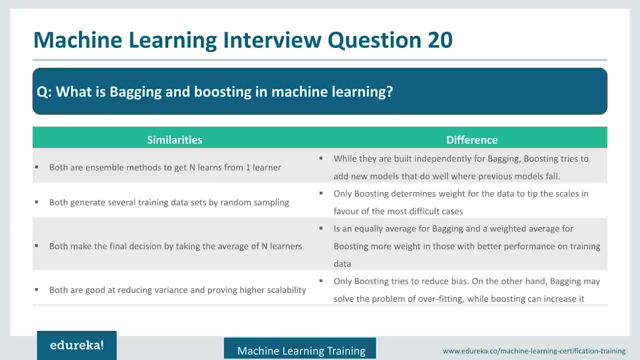 So in the case of classification, you try to take the class which is coming at the highest. if you're training a hundred models and you have a binary classification, assume that out of hundred models, if 80 models are predicting that your class 1 should be there and 20 models are predicting your, 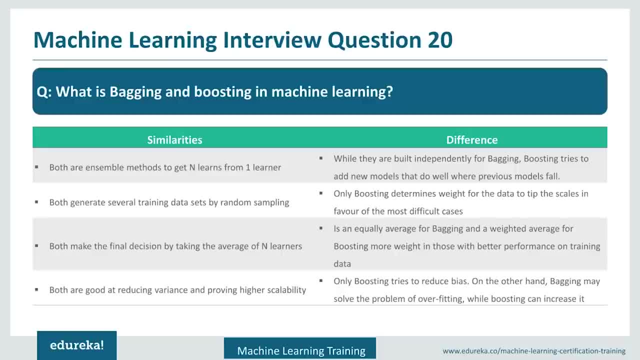 class 2 should be there. Then in ensemble, class 1 would be selected as output. In the case of regression, it is like you're trying to average all the outputs, as it's a continuous sequence. So in the case of regression, it is like you're trying to. 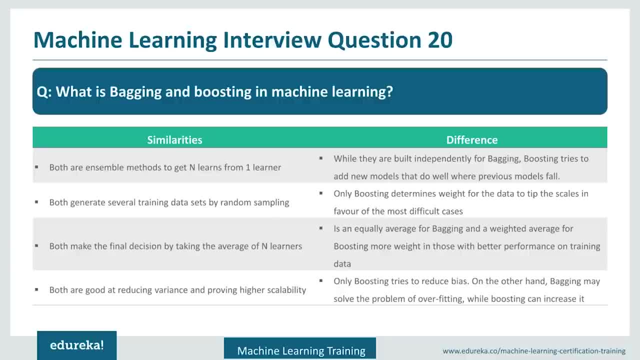 average all the outputs as it's a continuous sequence. So in the case of data, you try to aggregate all the output from the different models. So both are good at reducing the variance. So, as both are good at reducing the variance, as they are trying to learn different models, they reduce the overfitting of. 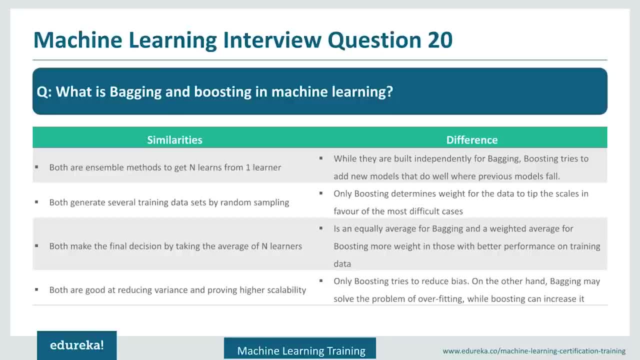 your data and, in effect, they also reduce the variance which is available within that model. So, as part of the differences boosting what it does is it tries to learn different weak learners is different samples are created. So in the case of regression, it is like you're trying to 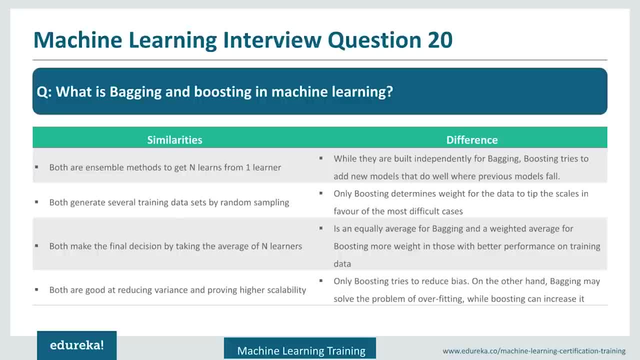 average all the cases. So, as part of the differences, boosting what it does is it tries to learn different weak learners- is different samples are created. So in the case of regression, it's like you're trying to achieve better performance. So, in the case of 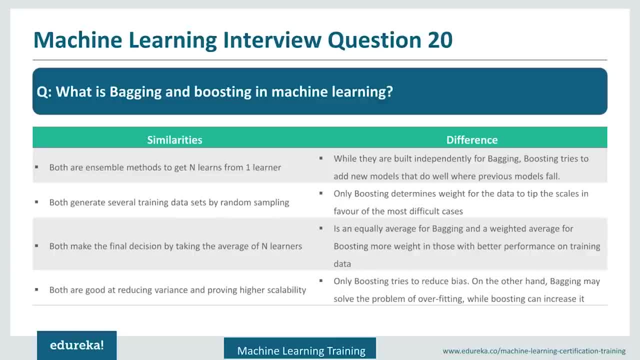 Lawrence & Faulkner, we will discuss wonderful machines. So in the case of regression, eachёre sample will gain value, is expected to become a better academic model And from this research hypothesis so far my grandchildren is taken to much view results and Past- steals in favour of the Nexus model. 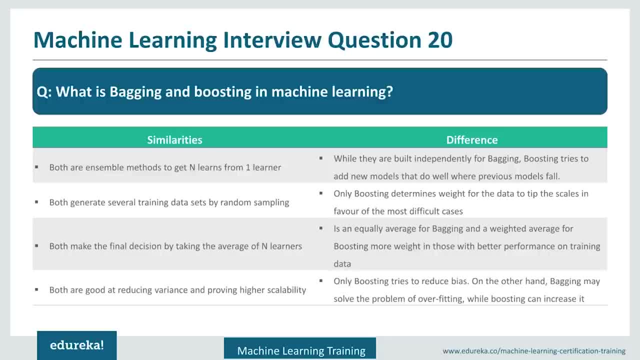 This new model has few tricks behind it, and the first trick is the hidden quelle's in the other model. This will be gone. treat the case. or the latest model: only hidden quelle's moving. it tries to change their weight and create a new model so that the new 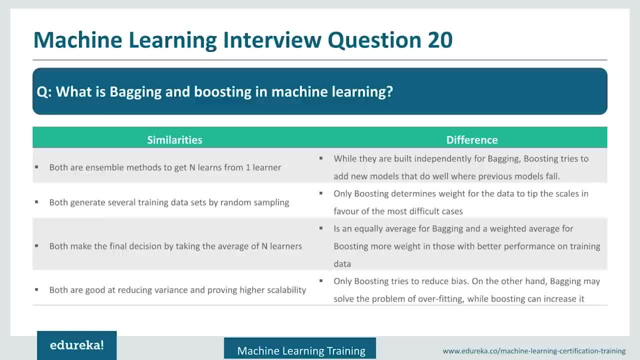 model will give more weightage to the ones which are misclassified in the previous model. so with this it keeps on improving itself. bagging gives equal weightage to each models output while creating ensemble output of your model, whereas boosting gives a difference weightage to each model, as each model is. 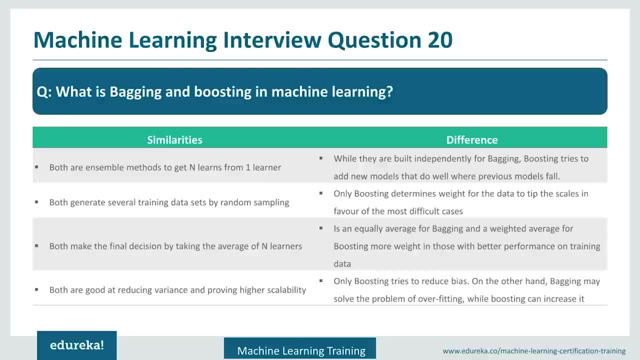 the improved version of the previous one. they have a difference weightage and the data weights are also changed, as within the each bagging model, so your weightage is also changed while you are aggregating the output of your boosting data. so as an ensemble model, both bagging and boosting- helps you to solve. 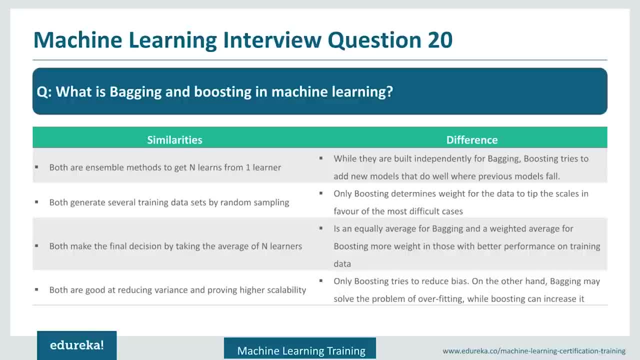 the problem of overfitting and, in effect, helping to reduce the variance. boosting tries to also reduce your bias, which is nothing but under fitting. as your keep on learning from this model, you will be able to reduce the variance of your the previous mistakes. you are getting better and better with the instances. 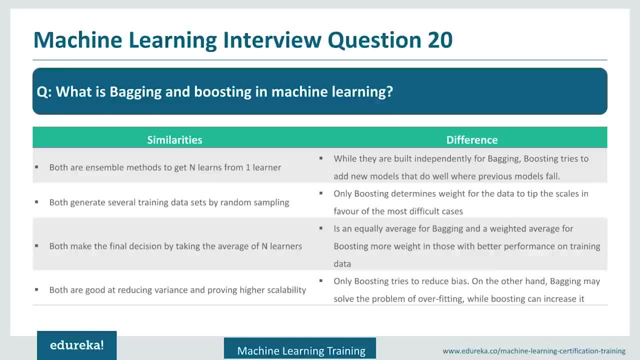 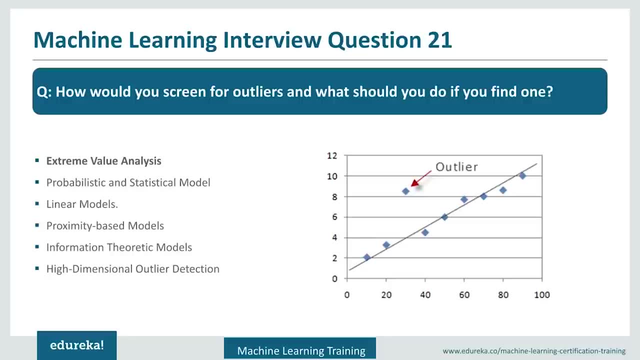 which are not much good, which is the bias. how do you screen for outliers and what should you do if you find one? in this case, your interviewer is interested to know, as how you give importance to the outliers, how you understand them and, when you find them, how we are trying to improve your models with the outliers. 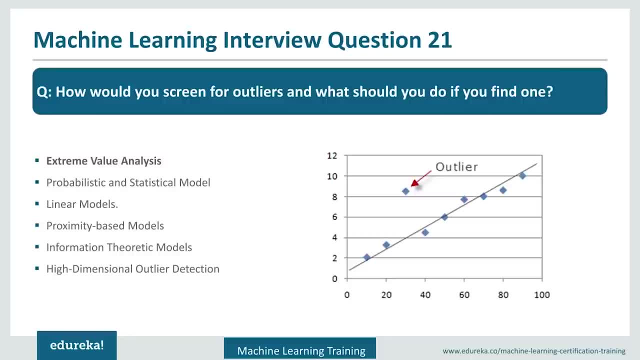 how you take your decisions once you know you get the outliers. so first thing you screen the outliers and then you get the outliers and then you get the outliers using different ways. so some of the ways are: one: is the box unlocked. so box plot really helps you to understand. when you plot the data you see that box. 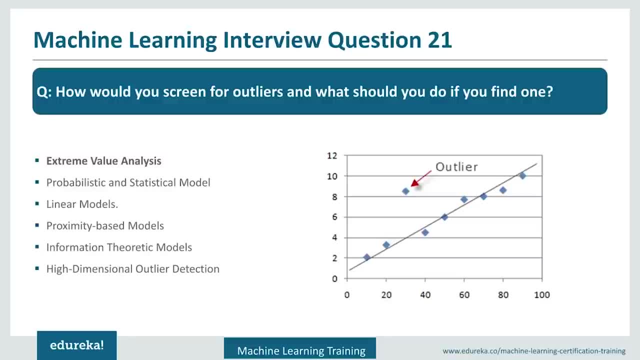 plot uses an formula of IQ are which is inter Quartile range multiplied by 1.5, plus your third quartile, minus your first quartile. this 1.5 x IQ R is added to the third quartile or to create the outliers on the top, and from the first quartile it is subtracted to create the 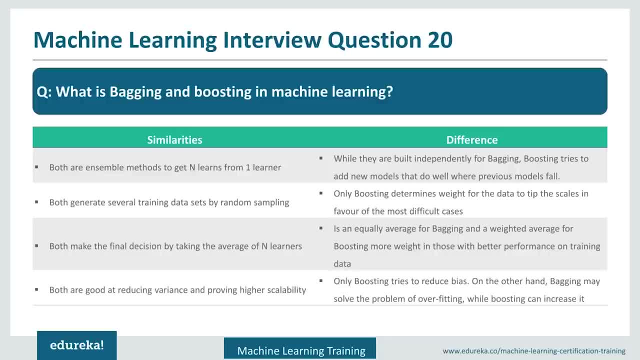 So boosting tries to wait the misclassified classes which were there in the previous model And so, as it Keeps on moving, it tries to change their weight and create a new model so that the new model will give more weightage to the ones which are misclassified in the previous model. 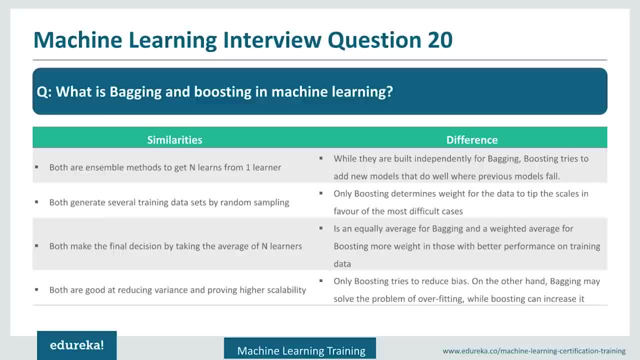 So with this, it keeps on improving itself. bagging gives equal weightage to each models output while creating ensemble output of your model, Whereas boosting gives a difference weightage to each model. as each model is a improved version of the previous one, They have a difference weightage and the data weights are also changed as within the each bagging model. 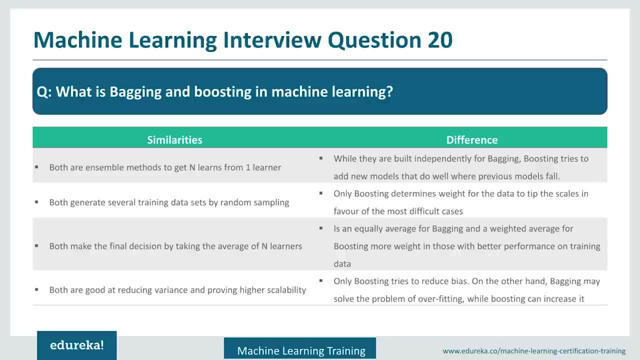 So your weightage is also changed while you're aggregating the output of your boosting data. So, as an ensemble model, both bagging and boosting helps you to solve the problem of overfitting and, in effect, helping to reduce the variance. boosting tries to also reduce your bias, which is nothing but underfitting, as your keep on learning from the previous mistakes. 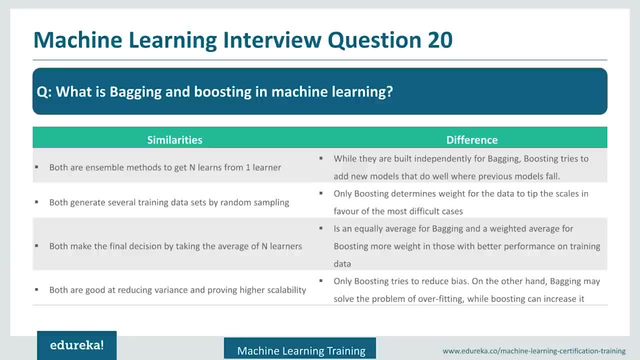 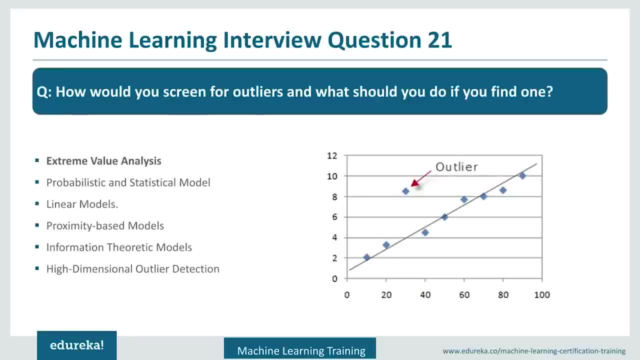 You're getting better And better with the instances which are not much good, which is the bias. How do you screen for outliers and what should you do if you find one? In this case, your interviewer is interested to know, as how you give importance to the outliers, how you understand them and when you find them, how we are trying to improve your models with the outliers- how you take your decisions once you know you get the outliers. 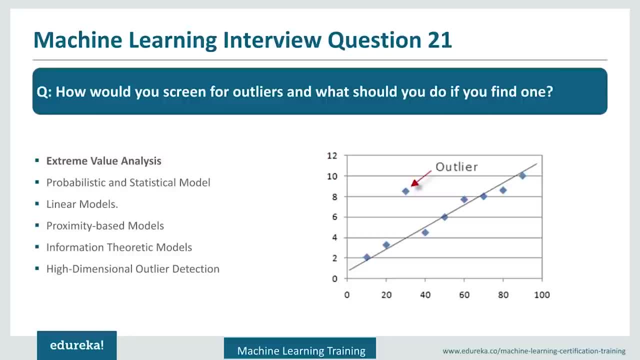 So, first thing, you screen the outliers using different ways. So Some of the ways are: one is the box plot. So box plot really helps you to understand. when you plot the data, you see that box plot uses an formula of IQR, which is interquartile range multiplied by 1.5, plus your third quartile, minus your first quartile. 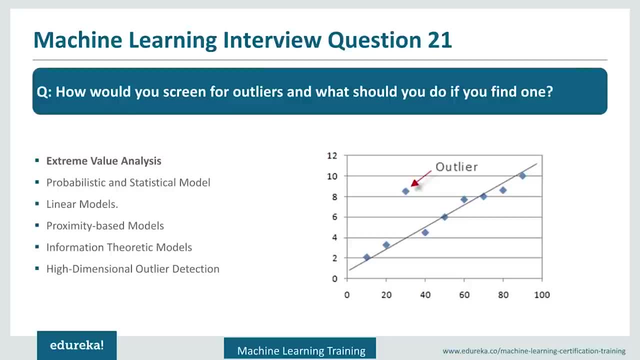 This 1.5, multiplied by IQR, is added to the third quartile to create the outliers on the top, and from the first quartile it is subtracted to create the outliers in the bottom line. So That is one way to screen the outliers using box plots. 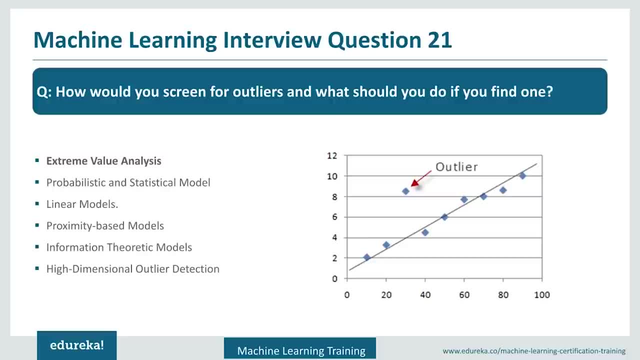 layers in the bottom line. so that is one way to screen the outliers using box plots. second is the probabilistic and statistical model. so, using the properties of different distribution models, such as the normal distribution, uh, the exponential distribution, the way your data follows it, you can see if your model is following those distributions or not and the cases where it is. 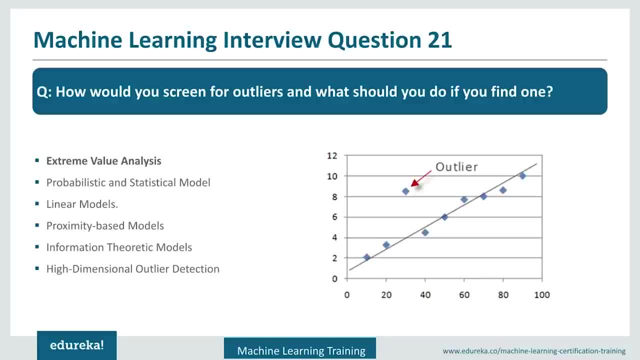 following very outside boundaries of your distribution. you can treat them as outliers. third is the linear models. so with the linear models you can try to see, as for example in the time series linear model. so when in the time series linear model, when you are learning the data, 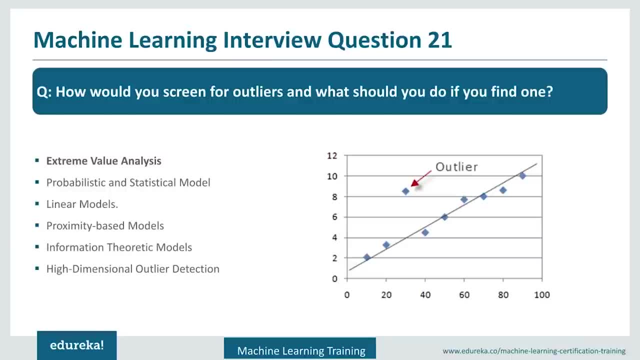 whenever a new outlier comes in, you will try to screen those. for the linear models, such as the logistic regression, you can try to flag them, uh, pre-hand, as okay, these are the outliers. flag them as one. these are the non-outlier. flag them as zero and your model will try to learn which are the. 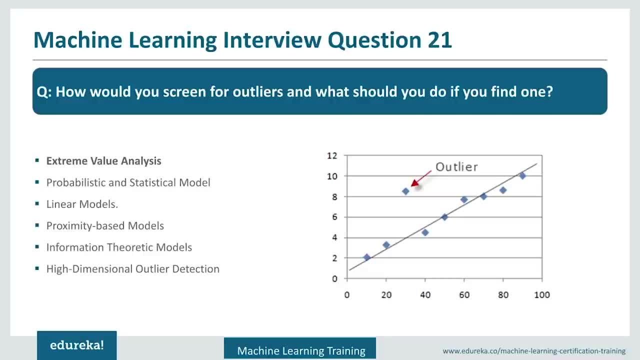 outliers and which are not, and in future you can use those models to screen your outliers within the data. and the last is the proximity based models. so proximity based models is like k-means clustering, so you use the k-means clustering to create a clusters within. 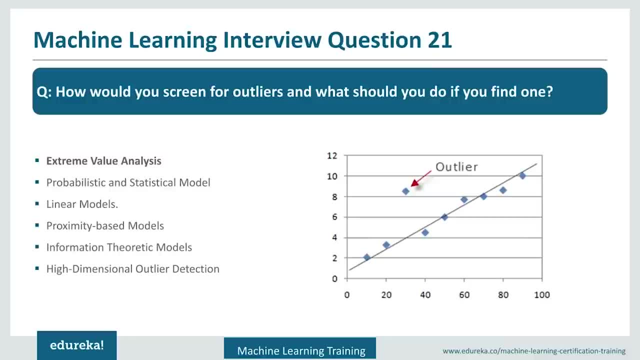 your data and the ones who fall outside of your clusters or outliers, will form themselves their own cluster and you will see that you will have your classified versions of your outliers. so, that is, with the proximity based model, how do you handle these outliers? you have to take a decision very carefully in this case, and how. 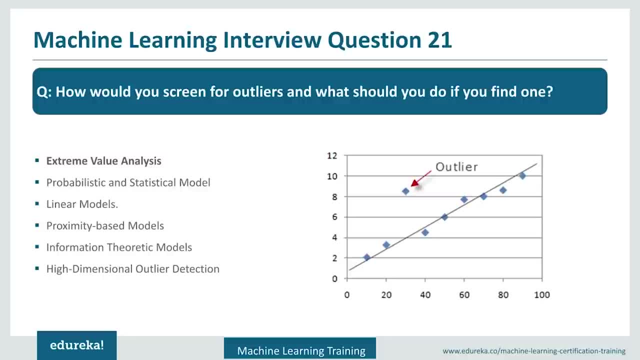 important are these outliers to your data, and when you have a very high data and you can risk dropping those outliers, then you can go on with that or you can cap your data using the percentile. so mostly what people do is they use the 99 percentile or 95 percentile, so whatever the 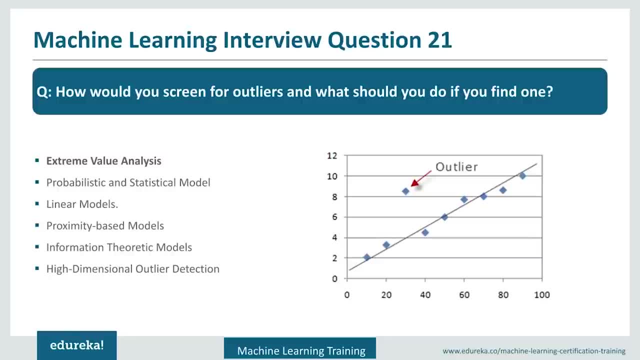 values are above those percentiles, your outlines are capped to those, so your outlines will get a little bit less impressive. um, you use this as well, so you can consider it as a Scanner, but you can use it in your project. so the last option is impute, based on some rules. 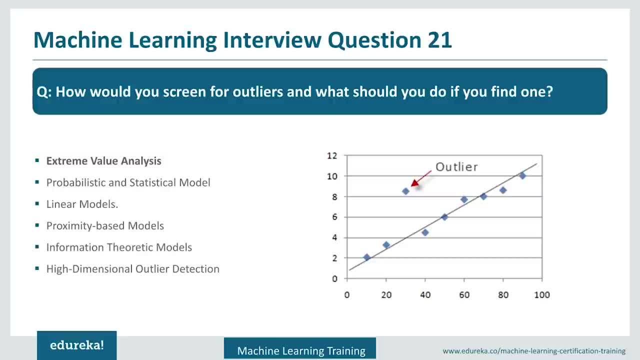 Second is the probabilistic and statistical model. So, using the properties of different distribution models, such as the normal distribution, the exponential distribution, the way your data follows it, You can see if your model is following those distributions or not and the cases where it is falling very outside boundaries of your distribution. 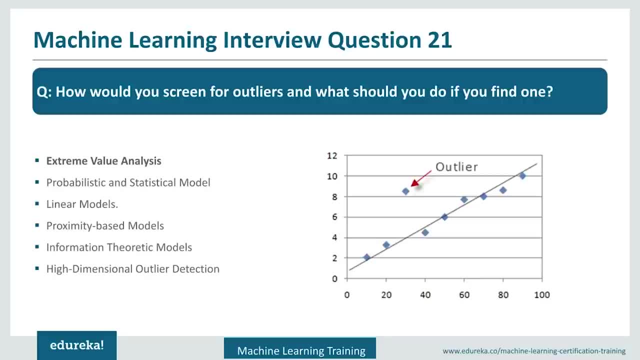 You can treat them as the outliers. third is the linear models. So with the linear models you can try to see, as For example in the time series linear model. so when in the time series linear model, when you're learning the data, whenever a new outlier comes in, you will try to screen those. for the linear models, such as the logistic regression, you can try to flag them pre hand as okay, these are the outliers, flag them as one, these are the non outliers, flag them as zero and your model will try to learn which are the outliers and which are not. and in future you can use those models to screen your outliers. 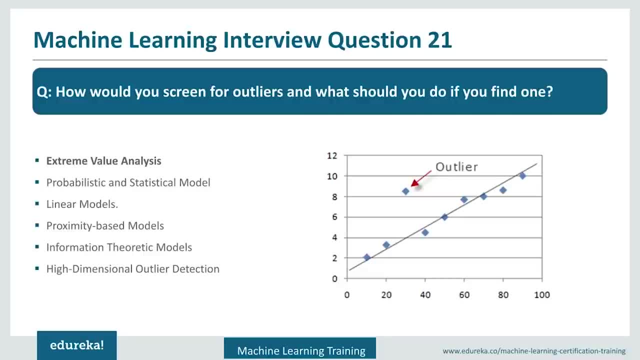 within the data. And the last is the proximity based models. So proximity based models is like k-means clustering, So you use the k-means clustering to create a clusters within your data and the ones who fall outside of your clusters or outliers, will form themselves their own cluster and you will see that you will have your classified versions of your outliers. 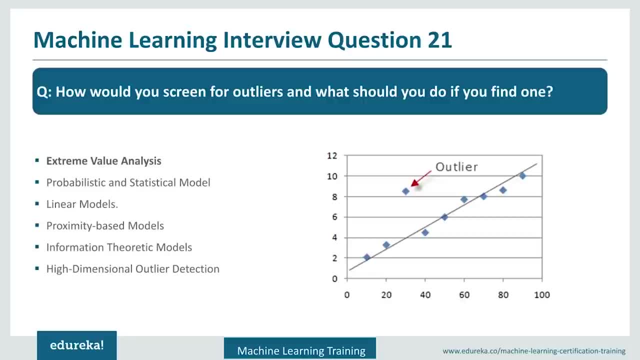 So, that is, with the proximity based models, How do you handle these outliers? You have to take a decision Very carefully in this case, and how important are this outliers to your data? and when you have a very high data and you can risk dropping those outliers, then you can go on with that or you can cap your data using the percentile. 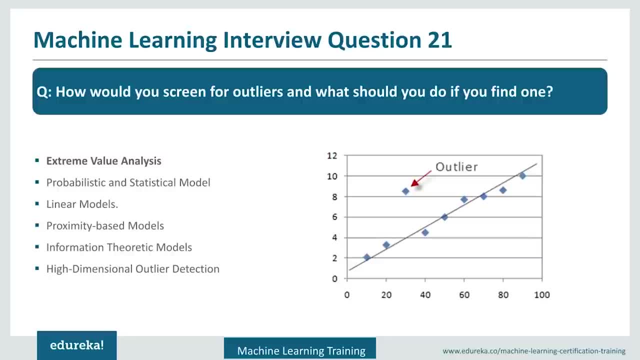 So mostly what people do is they use the 99 percentile or 95 percentile. So whatever the values are above those percentiles, your outliers are capped to those. so your outliers will get reduced. The last option is impute based on some rules. So based on some business rules or the data exploration that you do, using those, you can impute your outliers so that you can go on with the model creation. 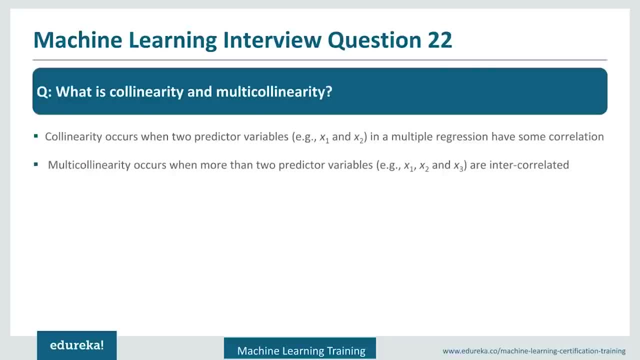 What is collinearity and multicollinearity? So this is one really interesting thing, as what happens in this case is so. collinearity occurs when you're trying to do a regression on a multi features and you see that your two of the predictors are correlated with each other. 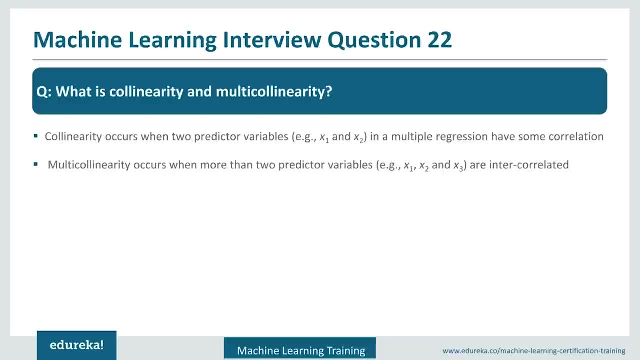 so, based on some business rules or the data exploration that you do, using those, you can impute your outliers so that you can go on with the model creation. what is collinearity and multicollinearity? so this is one really interesting thing, as what happens in this cases, so called in 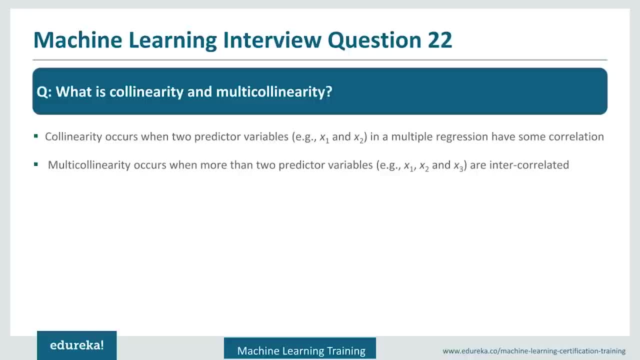 it occurs when you're trying to do a regression on a multi features and you see that your two of the with each other. for example, let's assume you have a date of birth and the age, so when you have both of this, your date of birth and age is always going to be correlated with each other. so in those cases, 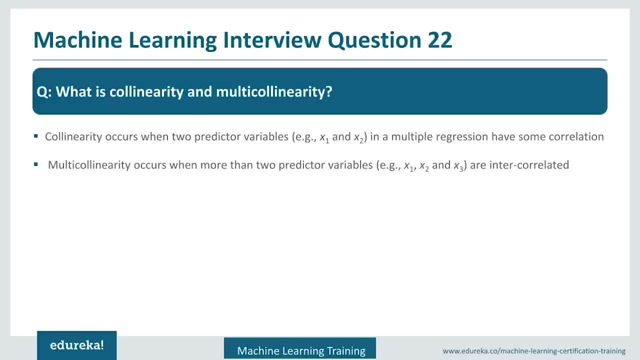 these two features are part of collinearity within the regression. multi-collinearity is something which occurs when you have more than two variables which are correlated with each other. so we can extend the previous example, which is: we have the age, we have the year on which he was born on. 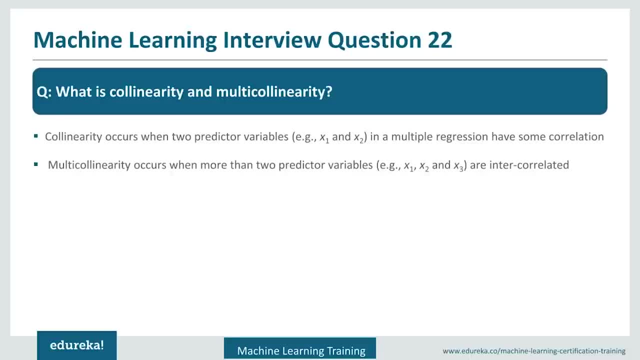 and the class that he is on currently. so, for example, if he is on fifth class, he is on seventh class, so those are also going to be correlated with each other. so in this case, we have three predictors which are correlated with each other. so what do you understand by eigenvectors? and 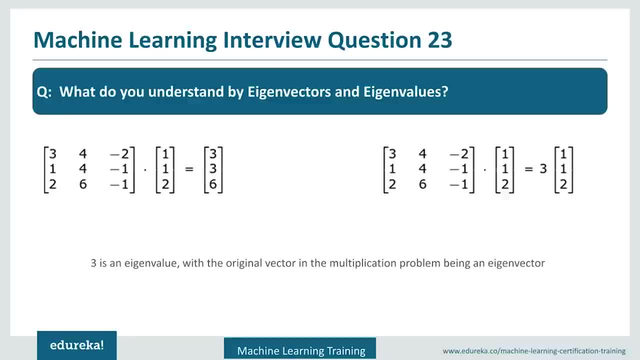 eigenvalues. so let's just see a bit of example to understand what is really happening in this. so in the left case, if you see, we have a square matrix which is being multiplied by a non-zero column matrix equal to the number of vectors, which is being multiplied by a non-zero column matrix. 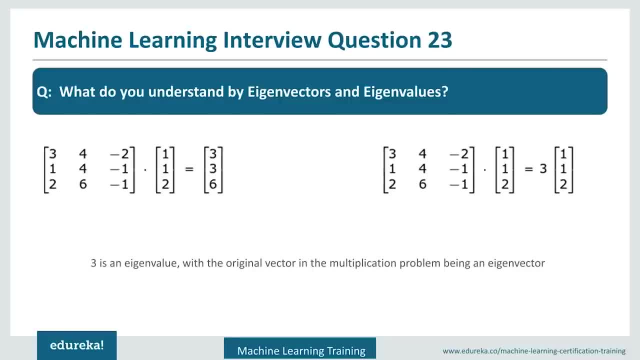 equal to, again, some a non-zero vector on the right side. if you see, we are getting an equation where our original square matrix is being replaced with three and we are still having the column vector. so we are able to represent the whole thing which is there on the left side to the right side by. 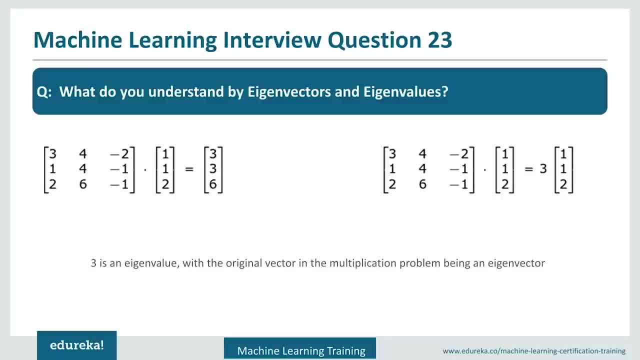 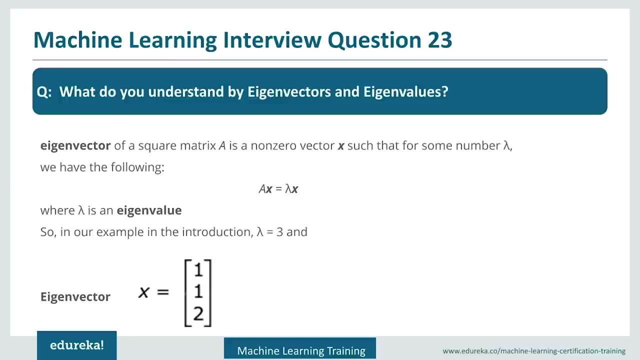 replacing the scalar. so the scalar in this case is called as the eigenvalue in the original vector and the multiplication that we are doing, the second vector is called as the eigenvector. so let's see the mathematical definition for this. if you see this equation, ax is equal to lambda x, so in this 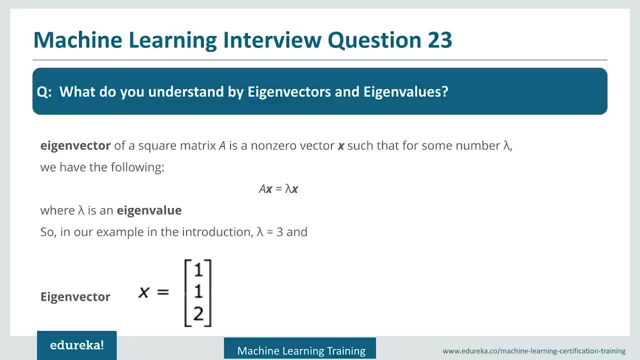 case, eigenvector of your square matrix a is a non-zero vector x, such that for sub number lambda we have this equation. so in this case we have this: square matrix a multiplied by our eigenvector gives us a lambda multiplied by eigenvector. so we are getting a scaled down version of the scalar. 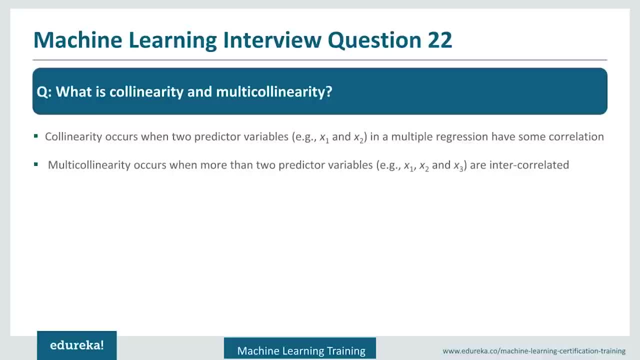 For example, let's assume you have a date of Birth and the age. So when you have both of this, your date of birth and age is always going to be correlated with each other. So in those cases, these two features are part of collinearity. within the regression, multi collinearity is something which occurs when you have more than two variables which are correlated with each other. 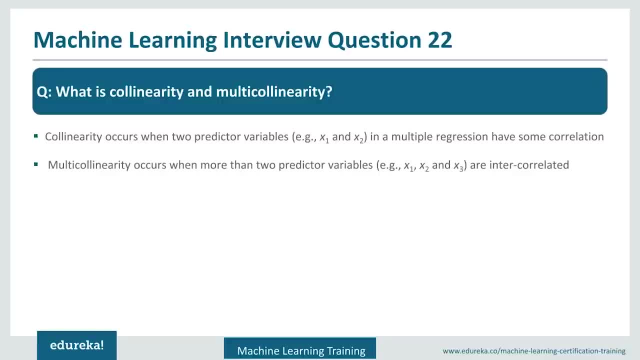 So we can extend the previous example, which is we have the age, we have the year on which he was born on and the class that he is on currently. So, for example, if he is on Fifth class is on seventh class. So those are also going to be correlated with each other. 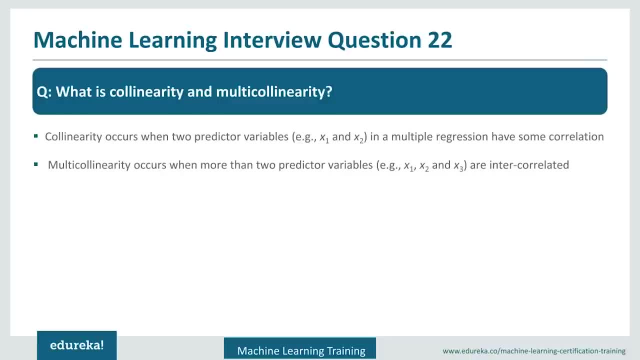 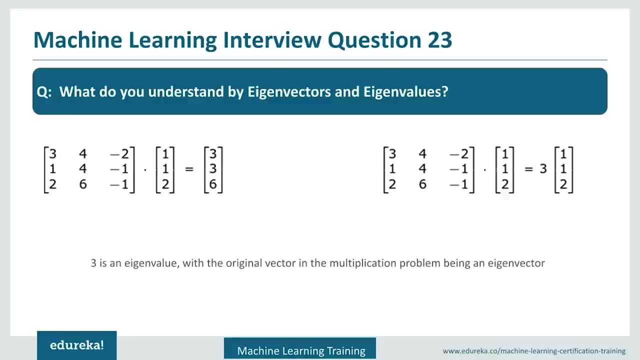 So in this case, we have three predictors which are correlated with each other. So what do you understand by eigenvectors and eigenvalues? So let's just see a bit of example to understand what is really happening in this. So in the left case, 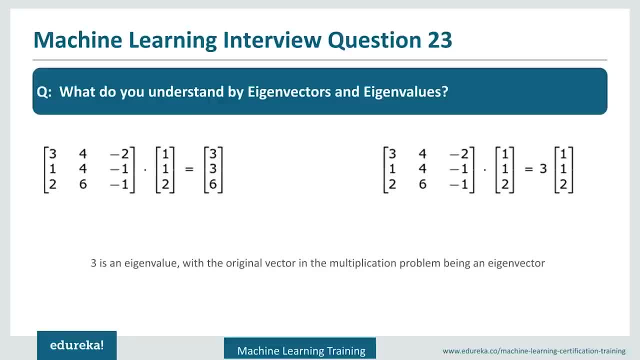 if you see, we have a square matrix which is being multiplied by a non-zero column matrix, equal to, again, some non-zero vector. on the right side, If you see, we are getting an equation where our original square matrix is being replaced with three and we are still having the column vector. 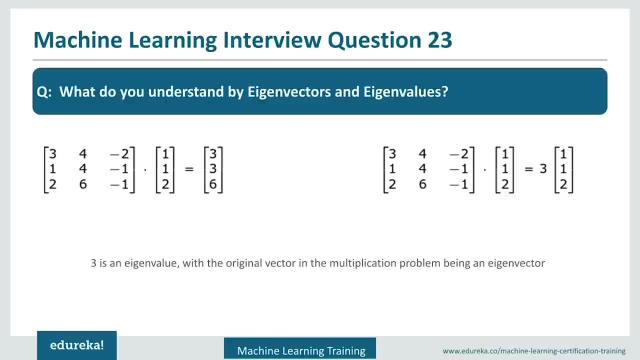 So we are able to represent the whole thing which is there on the left side to the right side by replacing the scalar. So the scalar in this case is called as the eigenvalue in the original vector and the multiplication that we are doing the second vector is called as the eigenvector. 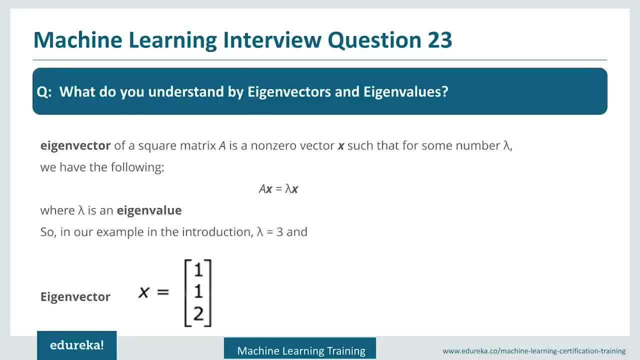 So let's see the mathematical definition for this. If you see this equation, ax is equal to lambda x. So in this case, eigenvector of your square matrix A is a non-zero vector x, such that for sub number lambda we have this equation. 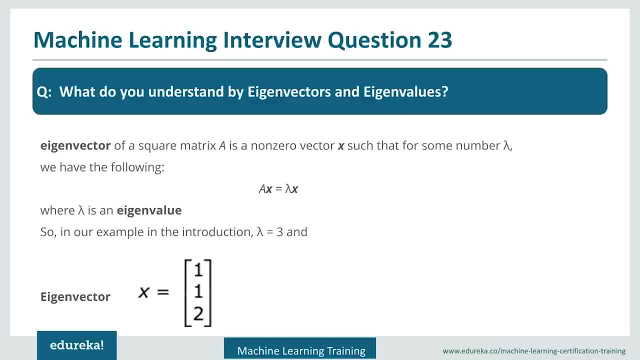 So in this case we have this square matrix: A multiplied by our eigenvector gives us a lambda multiplied by eigenvector. So we are getting a scaled-down version of the scalar square matrix as a scalar and which have its own applications. So 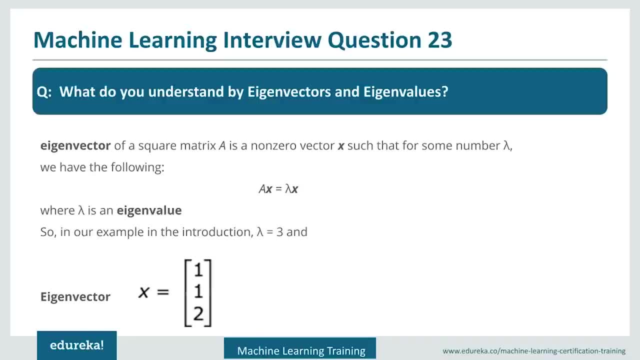 square matrix as a scalar and which has a non-zero vector. so we are getting a scaled down version of of the scalar square matrix as a logo. square matrix: so each column has a non-zero vector. so non-zero vector. then the number ofPlus or boundaries, areuito apartment should be equal to 1. how can you calculate both convergences? 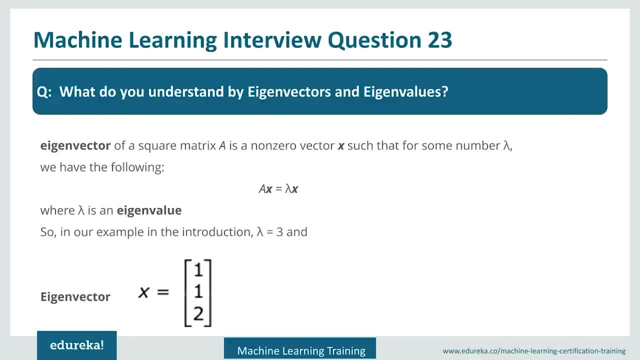 in a linear file and you could rely on. we can calculate the précis74 matrix on temperatura, given the shouting data of hexagon of the original matrix. we can calculate the corollary of responsibilities matrix without introducing a value. call in the way soon as your subscribers. 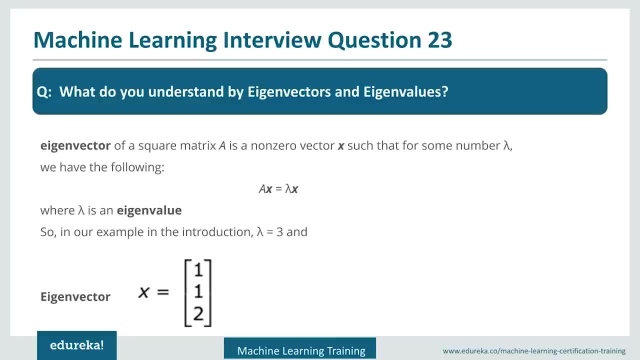 What this basically gives you is how much of your transformations are there and within the data, and these eigenvectors calculated from this correlation matrices can be used in the further algorithms called the PCA and the factor analysis, and these algorithms really helps you to reduce the dimensions which is there within your data. 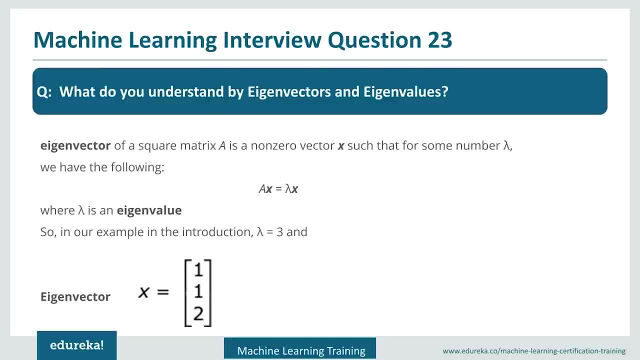 So that is from the point of data analysis. The other applications are eigenvectors, are the directions along which a particular relay transformation acts. So when you apply some linear transformation, this eigenvectors are actually giving you like in which direction those transformations are being applied. 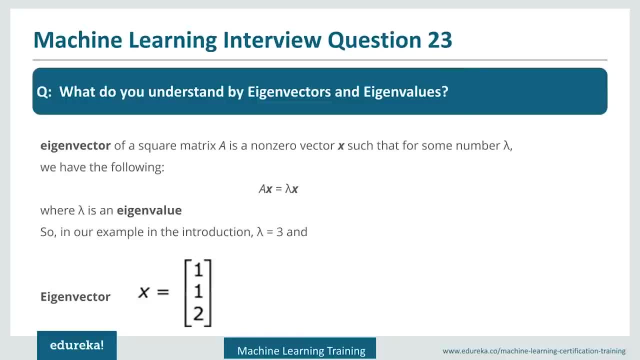 So this is like when you apply this transformation. what is the direction which is being there? It can also be used to do the compressions within the data. So eigenvalues and eigenvectors are also used in the image field, where images can be compressed. 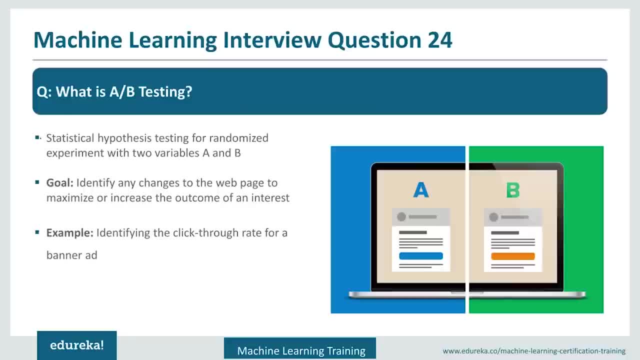 using those values. What is A-B testing? So A-B testing? A-B testing is a statistical hypothesis testing which tries to compare different cases. So in our cases we want to measure how different model performs as compared to each other. So assume that in production you have a model which is already running and tries to see. 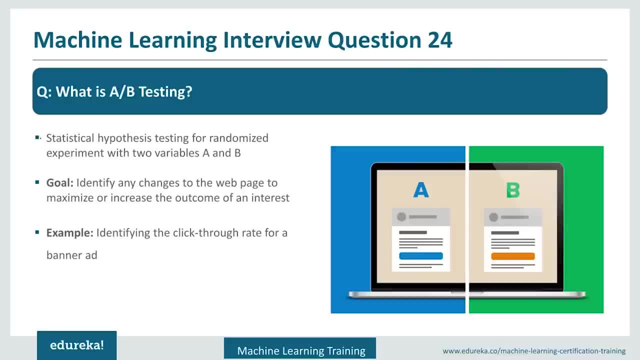 how your users are clicking through your products and they're buying those products. So your model basically predicts some recommendations of the products and captures like how, what is the ratio that once you recommend them and they buy it? So you introduce another model into the system which is just limited to few users and which 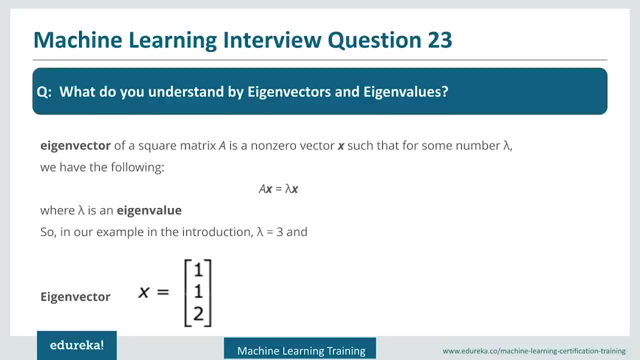 for example, how is this thing used? so a few of these use cases are: eigenvectors are used to understand the linear transformations which is there within your original square matrix. so in data analysis we visually calculate the eigenvectors for the correlation and covariance matrix of the original data. 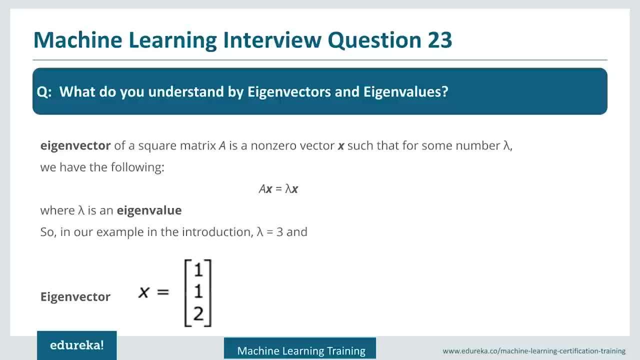 so, whenever we have any data, we can calculate the correlation matrices, covariance matrices, and we can calculate their eigenvectors from those matrices. what this basically gives you is how much of your transformations are there and within the data, and these eigenvectors calculated from this correlation matrices can be used in the further algorithms called the PCA and 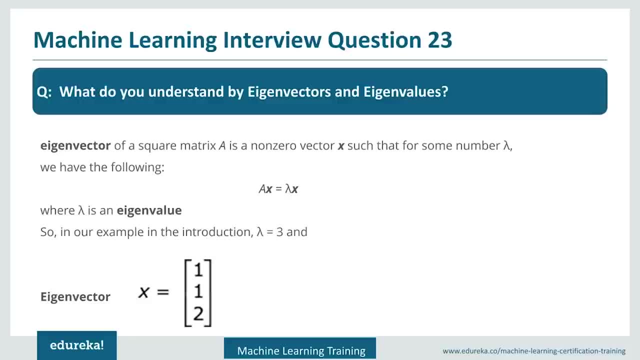 the factor analysis and these algorithms really helps you to reduce the dimensions which is there within your data. so that is from the point of data analysis. the other applications are eigenvectors are the directions along which a particular linear transformation acts. so that is from the point of data analysis. the other applications are: 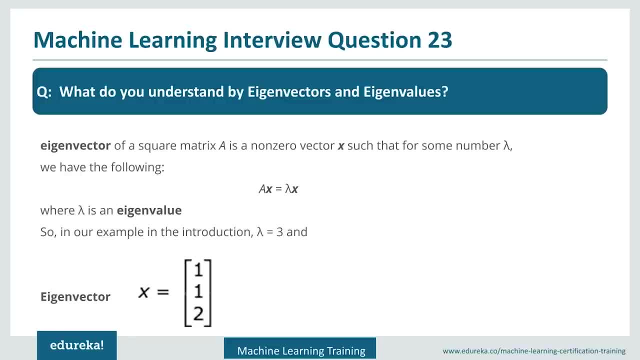 so when you apply some linear transformation, this eigenvectors are actually giving you like in which direction those transformations are being applied. so this is like: when you apply this transformation, what is the direction which is being there? it can also be used to do the compressions. 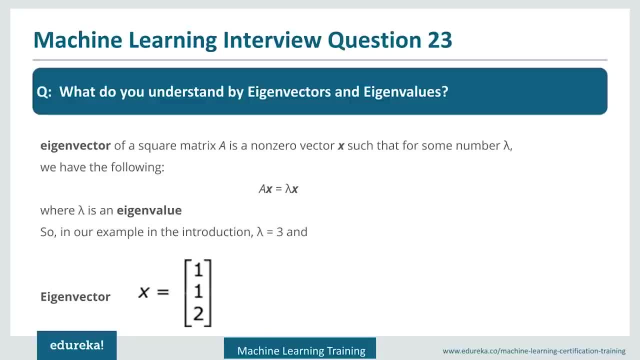 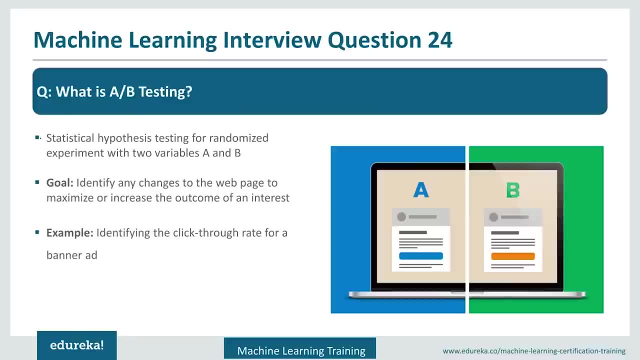 within the data. so eigenvalues and eigenvectors are also used in the image field, where images can be compressed using those values. what is a be testing? so a be testing is a statistical hypothesis testing which tries to compare different cases. so in our cases we want 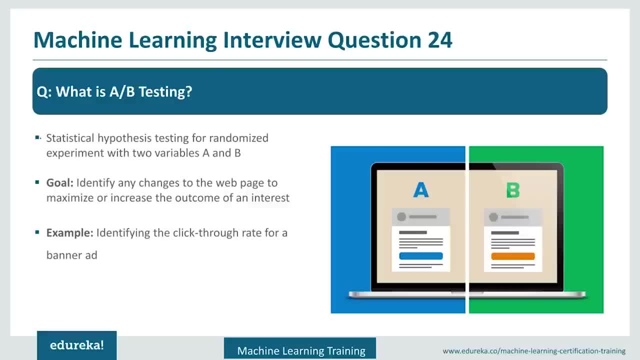 to measure how different model performs as compared to each other. so assume that in production you have a model which is already running and tries to see how your users are clicking through your products and they're buying those products. so your model basically predicts some recommendations of the 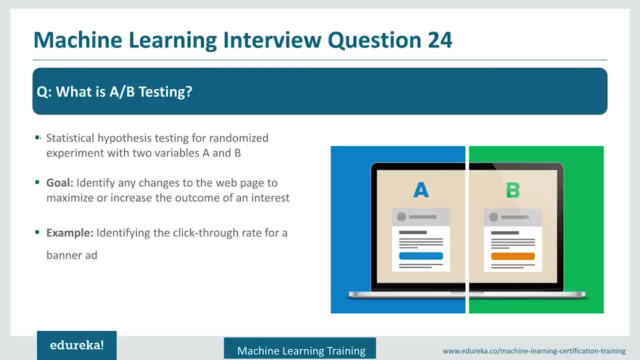 products and captures like how, what is the ratio that, once you recommend them and they buy it, you introduce an another model into the system, which is just limited to few users and which also does is it recommends your products and captures how many of them are actually buying those products. 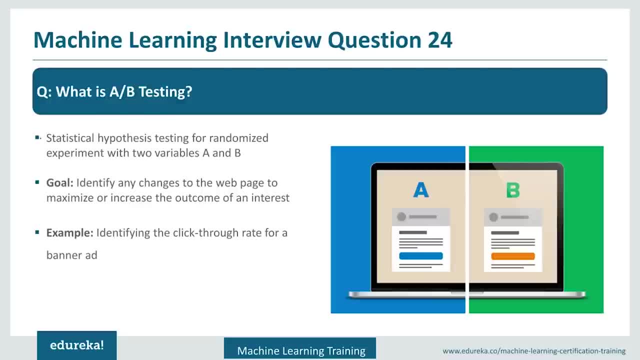 also does this. it recommends your products and captures how many of them are actually buying those products. Using some hypothesis testing, such as the TE test, ANOVA test and different tests, A-B testing tries to identify which model is better, which is trying to give you a better output. 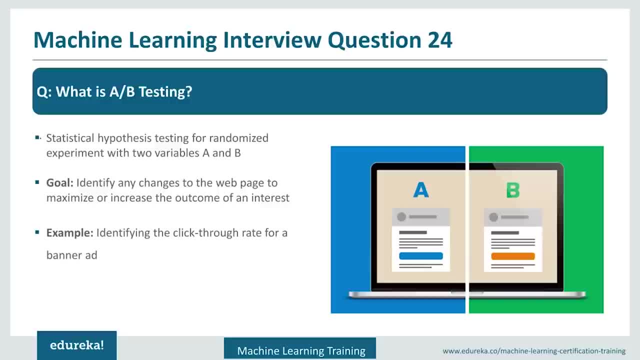 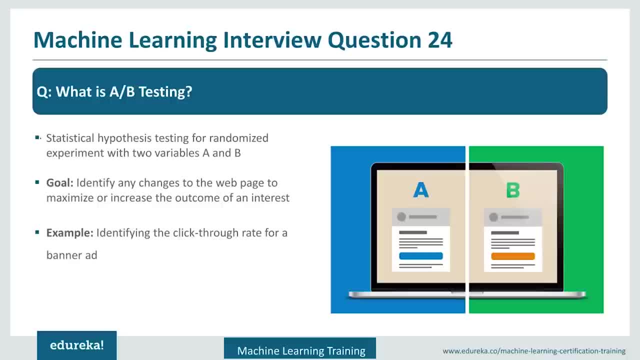 So you can give the examples to the interviewer, as in the cases where we want to test the model to different users and see how different functionalities are creating a better outcome and better revenues, And they use those things in the future. So what is cluster sampling? 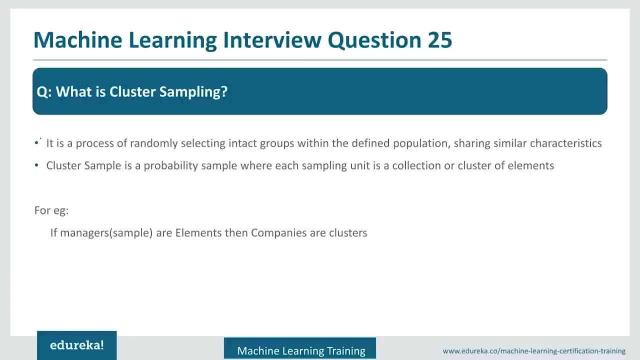 So when you have a population and within a population, you have different clusters available. So, for example, the previous example that we saw when we want to find out salaries of all the data scientists within India. So we have different clusters, like we have a cluster of Gurgaon. 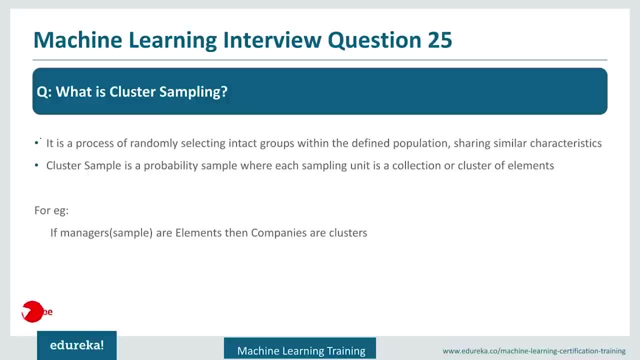 we have a cluster of Bangalore. we have a cluster of Mumbai, Pune, Hyderabad. These are the different clusters which we have, within which there are different data centers. When we try to randomly select those clusters for our analysis, that is called as the cluster sampling. 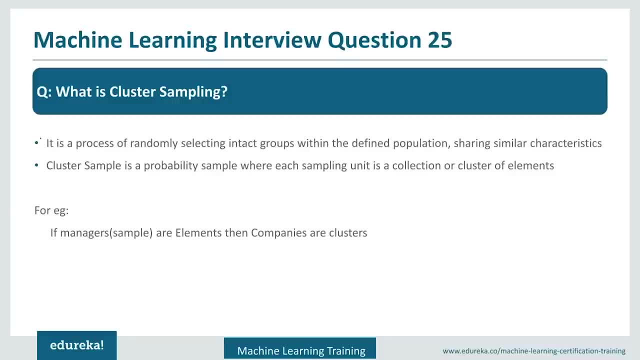 So in this case the sample is nothing but different clusters and we are trying to select those samples. So, for example, if managers are your samples, then companies are basically clusters And we do the clustering of those different companies when we select random clusters of these companies. 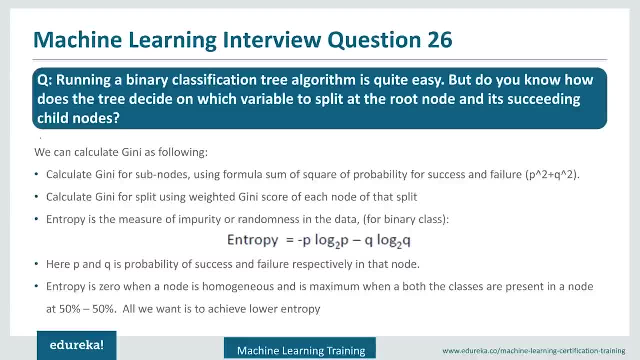 that is called as the cluster sampling. So running a binary classification tree algorithm is quite easy. But do you know how does the tree decide on which variable to split at the root node and its succeeding child node? So you can explain the things we have discussed already. 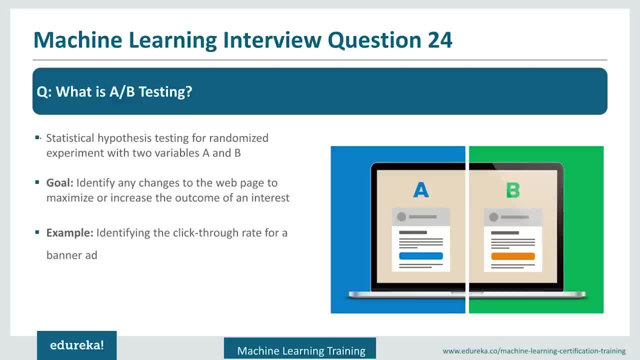 and using some hypothesis testing, such as the TE test, ANOVA test and different test A-B testing, tries to identify which model is better, which is trying to give you a better output in a comparison, So you can give the examples to the interviewer, as in the cases. 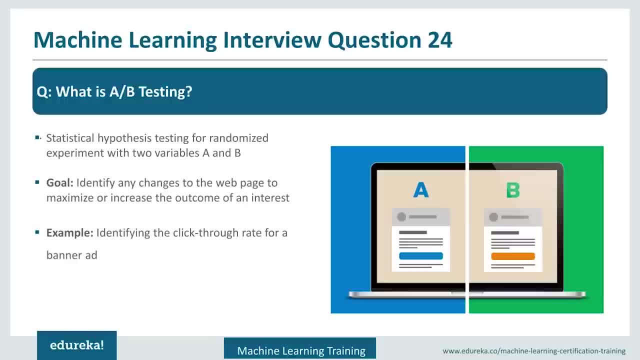 where we want to identify when a user clicks on the pages to increase the outcome of the interest. So some websites what they do? they try to introduce different functionalities to different users and see how different functionalities are creating a better outcome and better revenues and they use those things in a future. So what is cluster sampling? So when you have 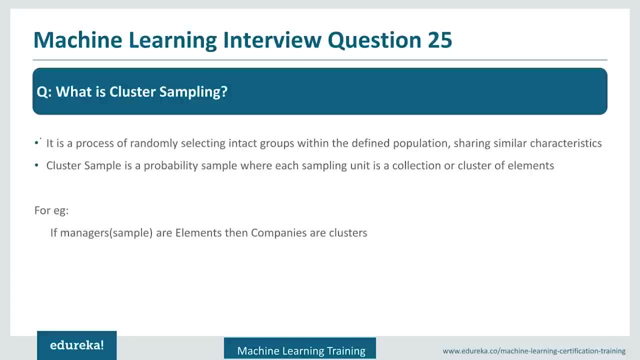 a population and within a population you have different clusters available. So, for example, the previous example that we saw when we want to create a cluster and we want to create a cluster. So in this case we want to find out salaries of all the data scientists within 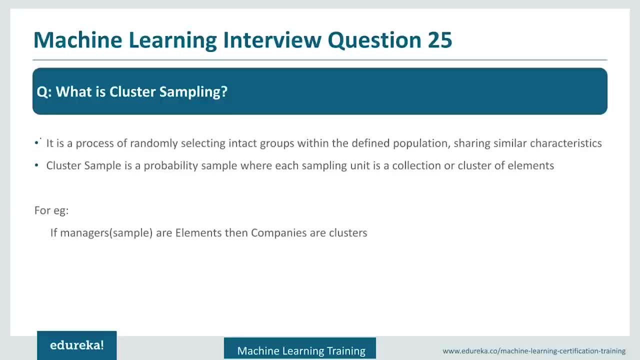 India. So we have different clusters, like we have a cluster of Gurgaon, we have a cluster of Bangalore, we have a cluster of Mumbai, Poornay, Hyderabad. These are the different clusters which we have, within which there are different data scientists. When we try 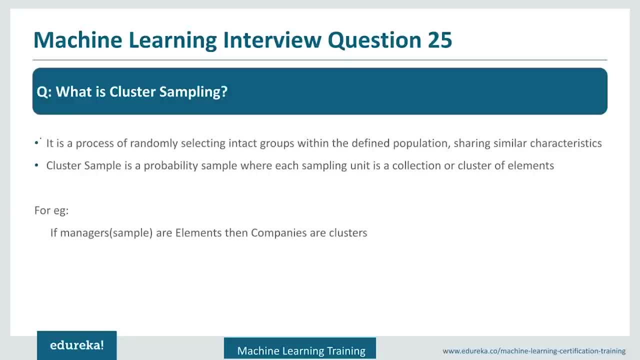 to randomly select those clusters for our analysis. that is called as the cluster sampling. So in this case the sample is nothing but different clusters and we are trying to select those samples. So, for example, if managers are your samples, then companies are basically clusters and 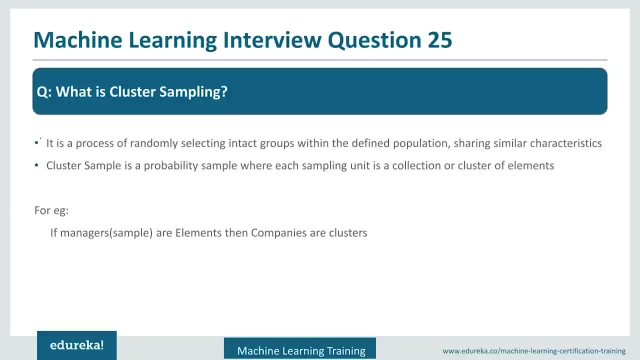 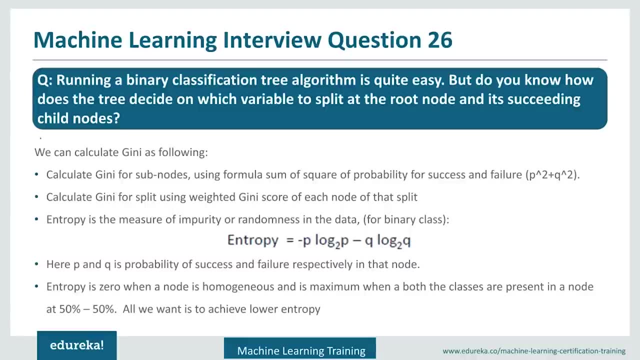 we do the clustering of this different company when we select random clusters of this companies. that is called as the cluster sampling. So running a binary classification tree algorithm is quite easy. But do you know how does the tree decide on which variable to split at the root node and 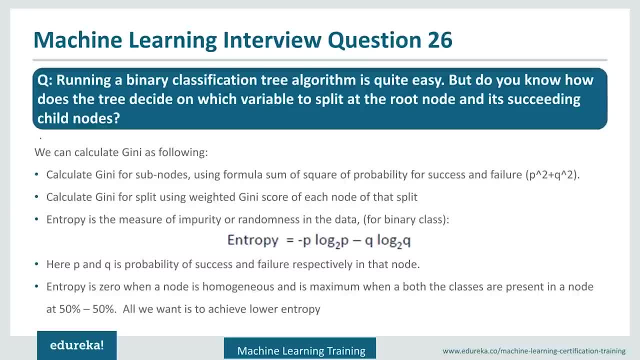 its succeeding child node. So you can explain the things we have discussed already about the Gini and the entropy parameters. So what Gini does is it calculates for sub nodes. what is the probability and success for each classes? and that is done by it squares the probabilities of success like p square. 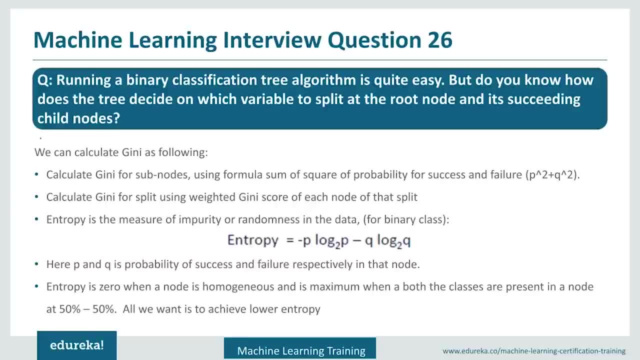 with the q square, which is the probability of success for each class and the probability of failure for other class. Once these probabilities are calculated, your weighted Gini score is calculated for each node. So whenever you have a lesser Gini score, you go with that feature for the splitting. 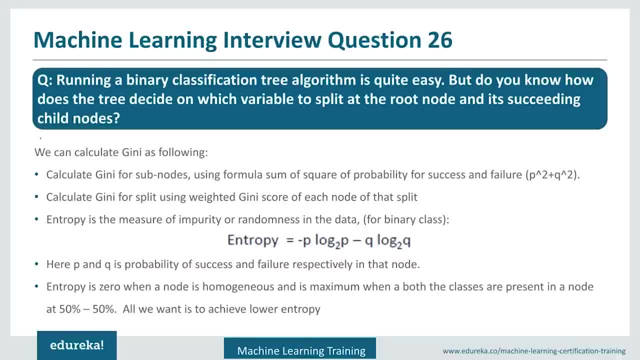 about the Gini and the entropy parameters. So what Gini does is it calculates for subnodes. what is the probability and success for each classes? And that is the Gini and the entropy parameters. So what Gini does is it calculates for subnodes. what is the probability and success for each classes? 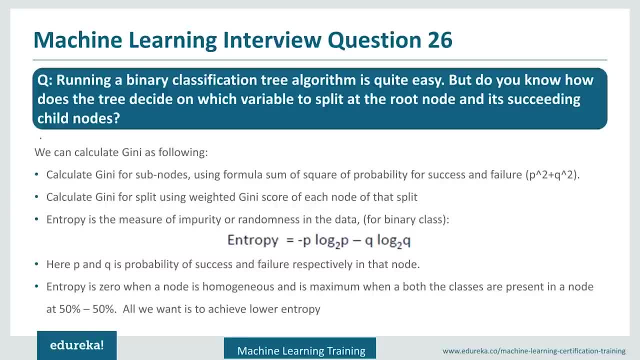 So what Gini does is it calculates for subnodes what is the probability and success for each classes and the probability of failure for other class. Once these probabilities are calculated, your weighted Gini score is calculated for each node. So whenever you have a lesser Gini score, 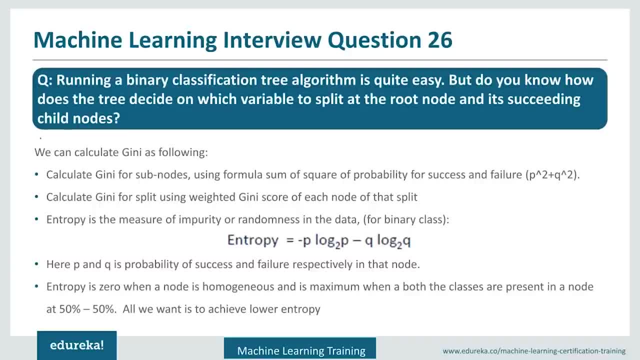 your weighted Gini score is calculated for each node, So whenever you have a lesser Gini score you go with that feature for the splitting of your nodes. Entropy is the measure of impurity or randomness within your data. It's like how misclassified your classes are within the class. 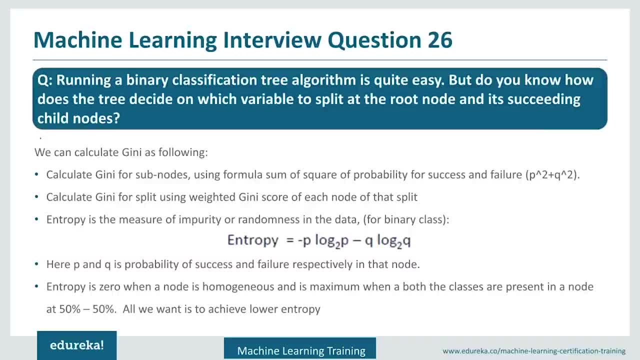 nodes. So it's for the binary classification. When you have the binary classification, we have the probability of success, we have the probability of failure. So for the positive class we have the probability of success and the other one we have the probability of failure. So we use the entropy. 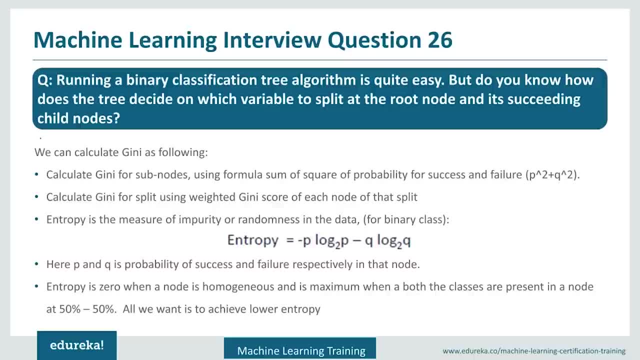 formula to calculate which one to split. So for whichever variable we have the lesser entropy, we go with the split of that node. So entropy is basically zero when a node is homogeneous. So when everything is within a single node and your node is completely pure, your entropy becomes. 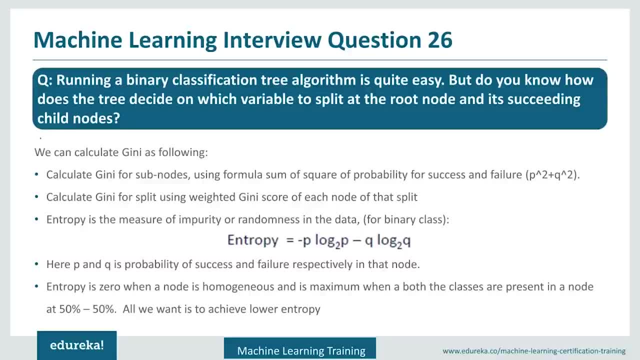 zero where a node completely contains a single class. When a node contains a 50- 50 percent of your classes, your class one is like if it is 100 rows and 50 of them are class one, 50 of them are class two. at that point your entropy value is highest. 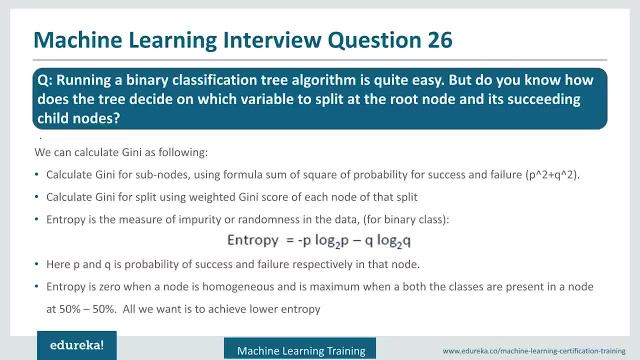 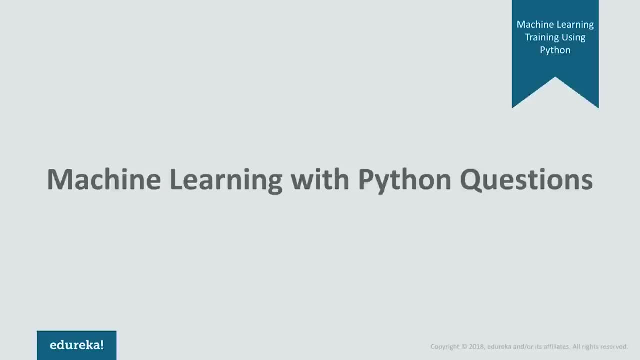 So the maximum value it will take when you have both the classes in the equal number within the nodes. The final agenda is to lower the Gini or the entropy, For whichever feature we have. the lower value go with the split of those for the current parent node. So now we are done with the core. 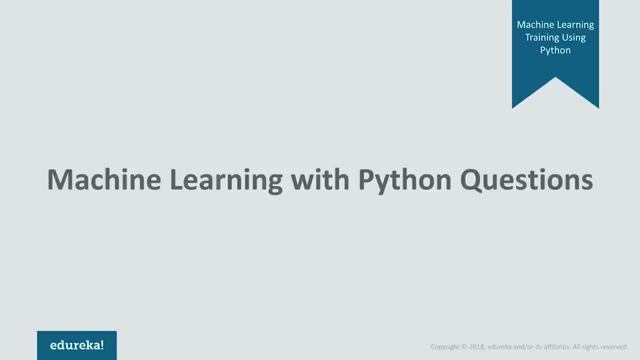 machine learning, which are mostly related to the theoretical aspects of the machine learning. Now we will start with the Python related questions with the machine learning, As machine learning can be done with different languages, So we will start with the Python related questions with the machine learning. 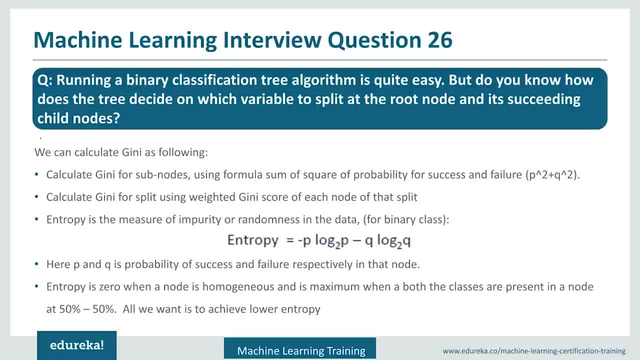 of your nodes. So entropy is the measure of impurity or randomness within your data. It is like how misclassified your classes are within the nodes. So it is for the binary classification. When you have the binary classification we have the probability of success. we have the 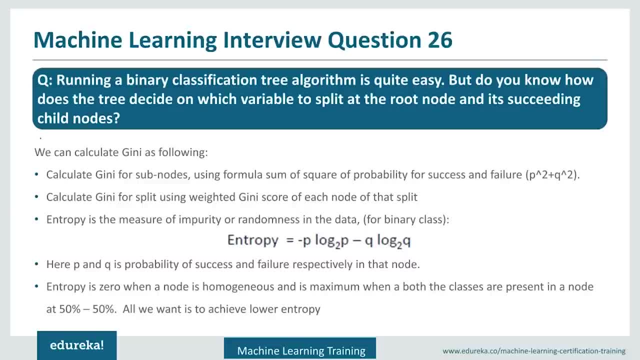 probability of failure. So for the positive class we have the probability of success and the other one we have the probability of failure. So we use the entropy formula to calculate which one to split. So for whichever variable we have the lesser entropy, we go with the split of that node. 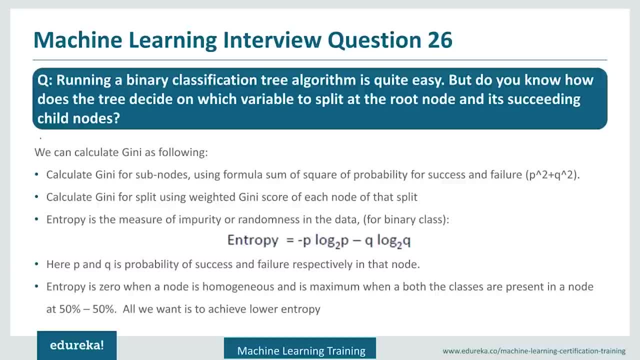 So entropy is basically zero when a node is homogeneous. So when everything is within a single node and your node is completely pure, your entropy becomes zero where a node completely contains a single class. When a node contains a 50-50 percent of your classes, your class one is like if it is a 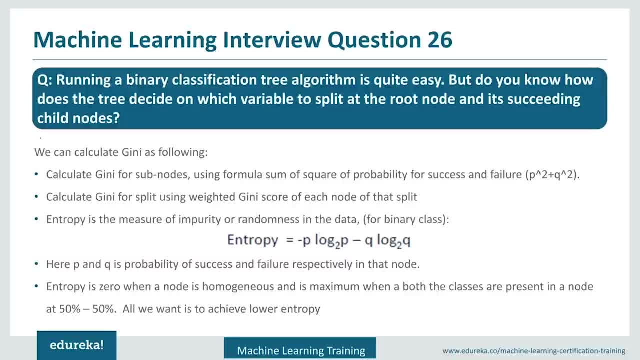 hundred rows and 50 of them are class one, 50 of them are class two. at that point your entropy value is highest, So the maximum value it will take when you have both the classes in an equal number within the nodes. The final agenda is to lower the Gini or the entropy. 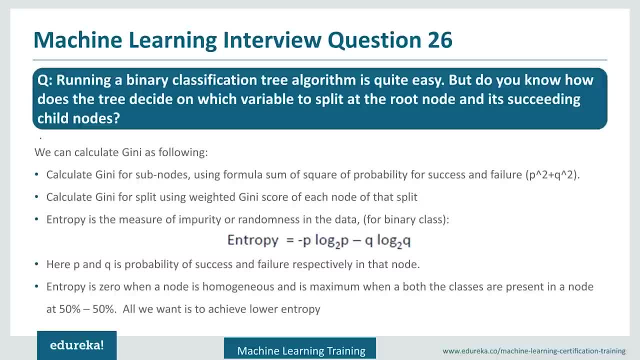 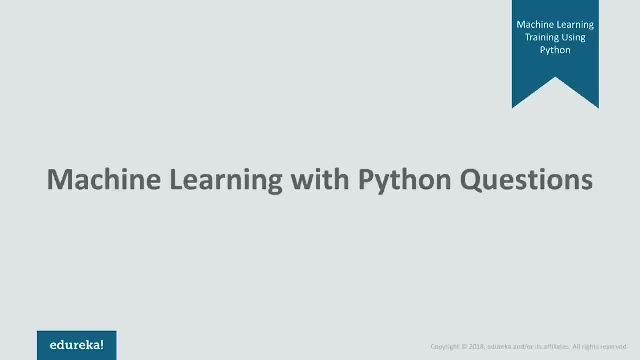 For whichever feature we have the lower value, go with the split of those for the current parent node. So now we are done with the core machine learning, which are mostly related to the theoretical aspects of the machine. Now we will start with the Python related questions with the machine learning. 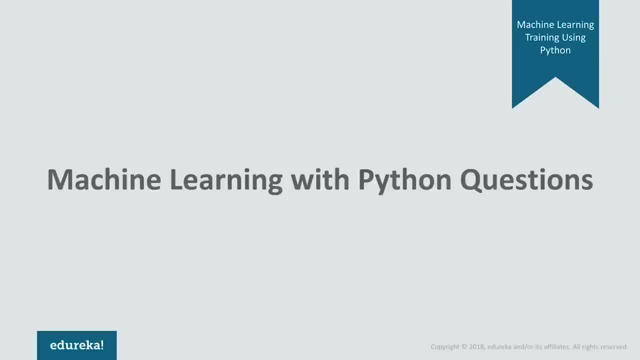 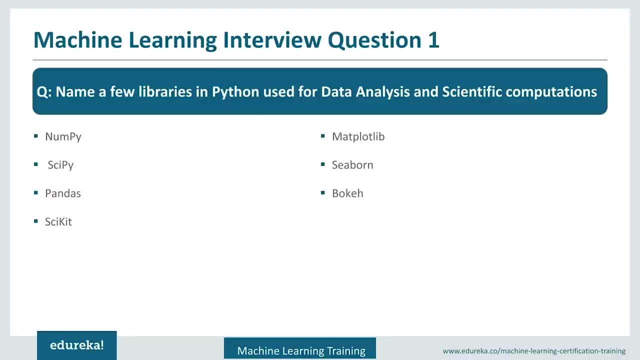 As machine learning can be done with different languages like R, Python, SAS, but currently we are more focusing on the Python and we will start with our practical questions which are there with the machine learning. So first question is: name a few libraries in Python used for data analysis and scientific 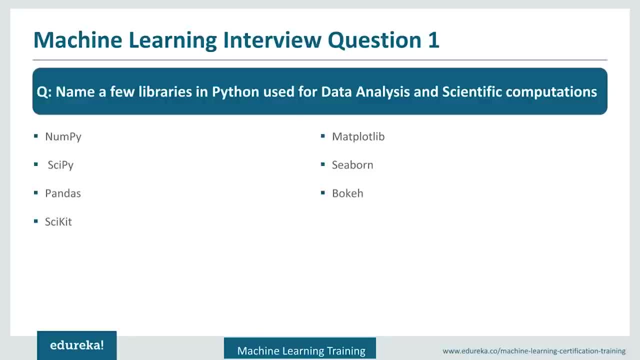 computations. In this case interview is trying to understand. So in the initial level he will try to understand. He will try to ask you these questions to gauge you if you really know about the core libraries which are used for the data analysis in the Python or not. 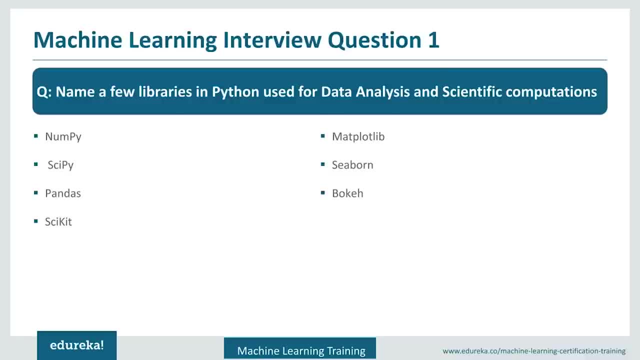 So the core libraries which are there within Python are NumPy, SciPy, Pandas and SkyKet. So first of all, NumPy. NumPy is a numerical library to deal with the data, So, as the name suggests, it is a numerical pie. 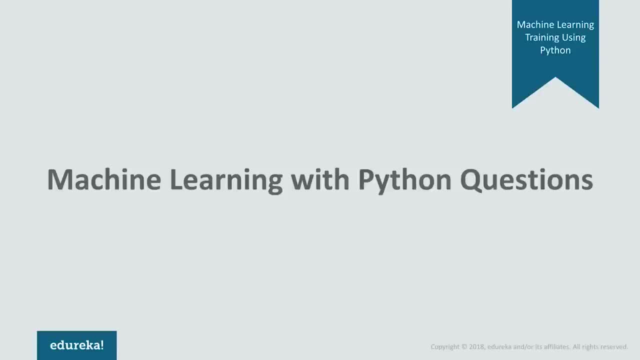 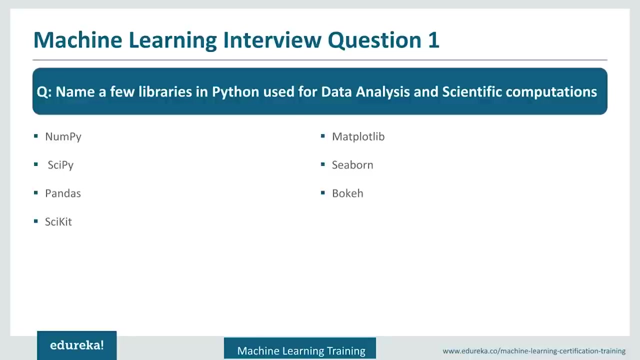 So we will start with the Python related questions with the machine learning. So first question is: named a few libraries in Python used for data analysis and scientific computations, In this case interviews is trying to understand, So in the initial level he will try to ask you these questions to guide you, if you really 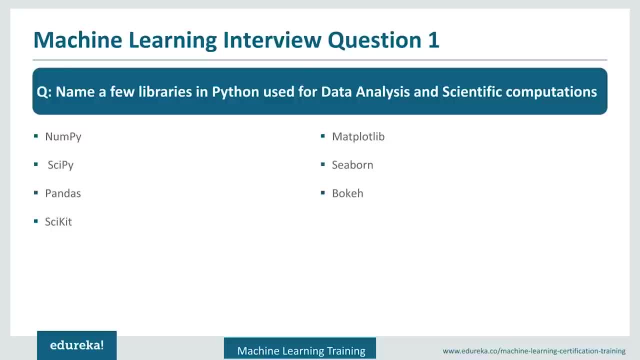 know about the code libraries which are used for the data analysis is in the python or not. so the core libraries which are there within python are numpy, scipy, pandas and skykit. so first of all, numpy. numpy is a numerical library to deal with the data, so, as the name suggests, it's a numerical pi, so it tries to deal with the numbers. so all the core. 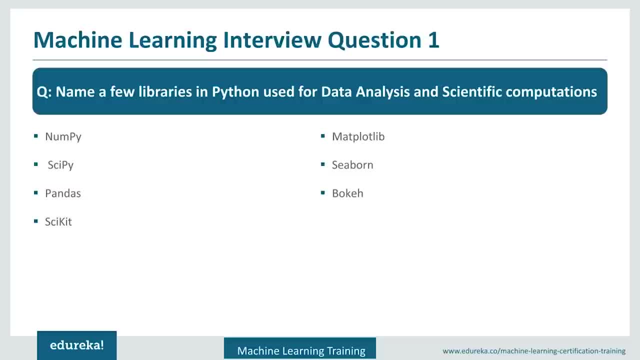 libraries such as the scipy panda. skykit uses numpy to store the data, so those are the core storage format for all the data in data analysis. so scipy, its full form, is basically scientific python. so it basically gives you a library to deal with all the different kind of mathematical. 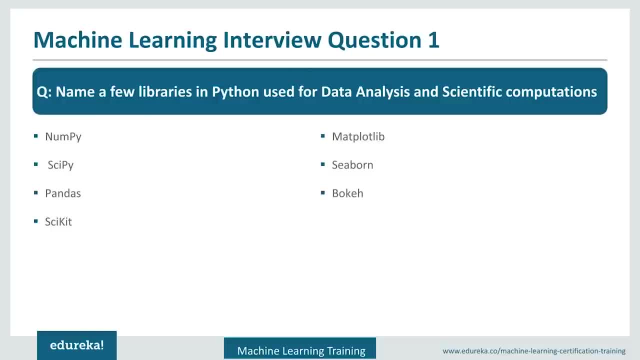 functions so you can do fourier transforms for the audio related data. you can go with the optimizations, you can go with the interpolation. so these are just a few examples. but all the mathematical related tasks you can go with the scipy and scipy uses, as we already discussed. 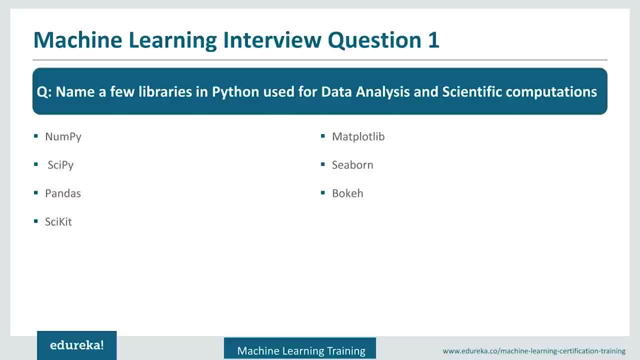 in a core numpy to store the data. so is a data analysis library again, where you can store the data in a tabular manner, which is called as a data frames, and data frames are very powerful function within pandas. so data from gives you a data manipulation access. you can access the csv, you can load the databases, you can load the. 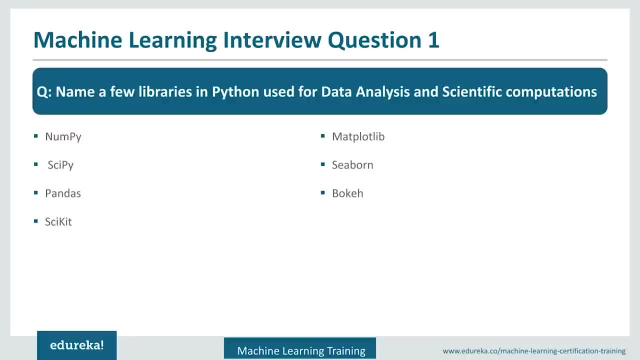 excel files and you can do your operations on top of it. you can do the aggregations, merging and all those kind of analysis related to the data you can do with the pandas. scikit is purely a machine learning library. what it gives you is access to the different 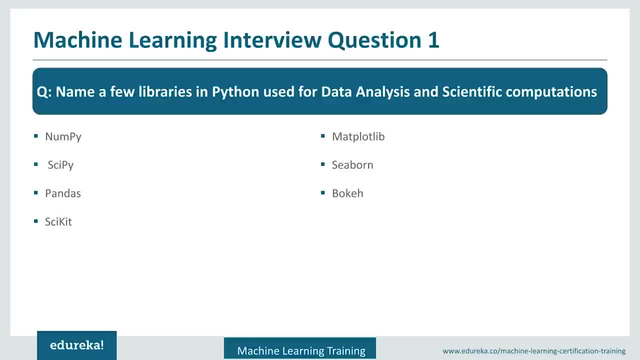 So it tries to deal with the numbers. So all the core libraries, such as the SciPy Pandas, SkyKet, uses NumPy to store the data, numpy to store the data. so those are the core storage format for all the data in. 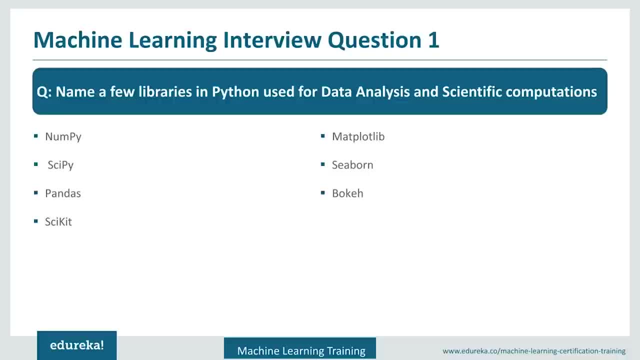 data analysis. so scipy, its full form is basically scientific Python. so it basically gives you a library to deal with all the different kind of mathematical functions. so you can do Fourier transform for the audio related data, you can go with the optimizations, you can go with the interpolation. so 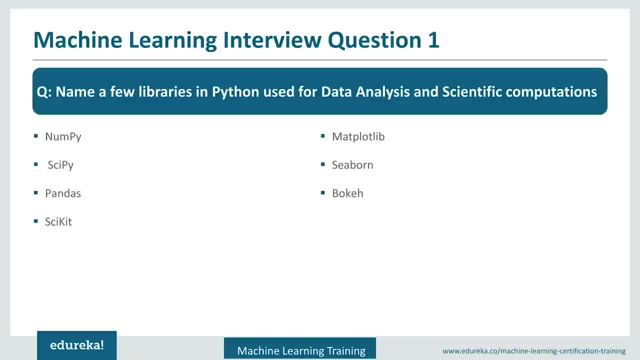 these are just a few examples but all the mathematical related tasks you can go with the scipy and scipy uses, as we already discussed, in a core numpy to store the data. so pandas is a data analysis library, again where you can store the data in a tabular manner which is called as a data frames and data. 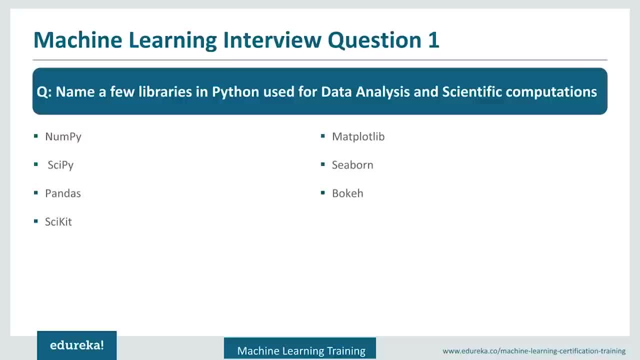 frames are very powerful function within pandas. so data from gives you a data manipulation access. you can access the CSV, you can load the databases, you can load the excel files and you can do your operations on top of it. you can do the aggregations, merging and all those kind of analysis related to the data. you can do with the. 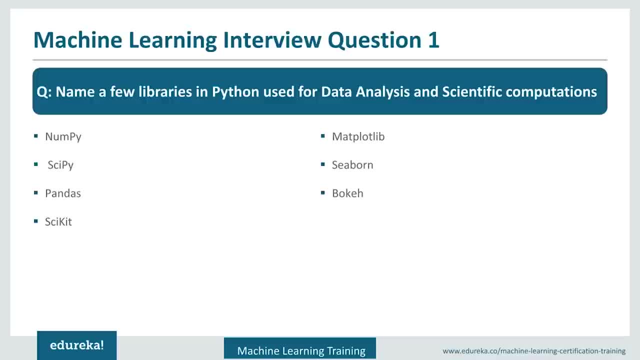 pandas psychic is purely a machine learning library. what it gives you is access to the different machine learning models you can use. so it contains a different components. it contains a pre-processing component where you can do the pre-processing of your data. it provides a library for that and it also 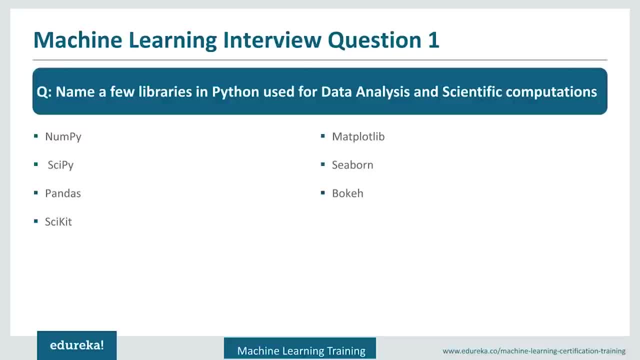 provides you a different modeling library where you can access all the core machine learning models. so on top of that we have matplotlib, which is a purely of data visualization tool. so with the matplotlib you can visualize your data in a very efficient manner and in a faster manner, and C bon is something which is built on. 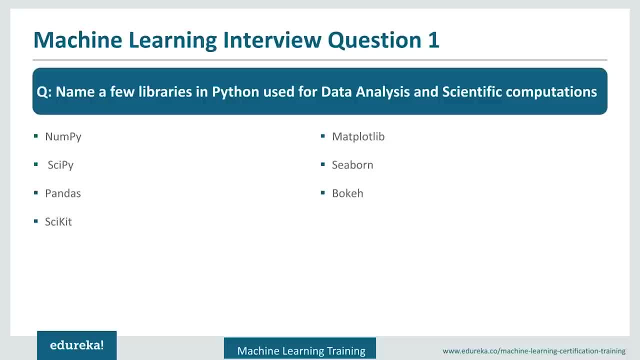 top of matplotlib and gives you a more better visualization of the data and gives you different new kinds of visualizations which are not there with the matplotlib. so you just can give you the detail you to the interviewer, just list them all and give a bit of the description about theuses and previews to understand the things that ability may or may. 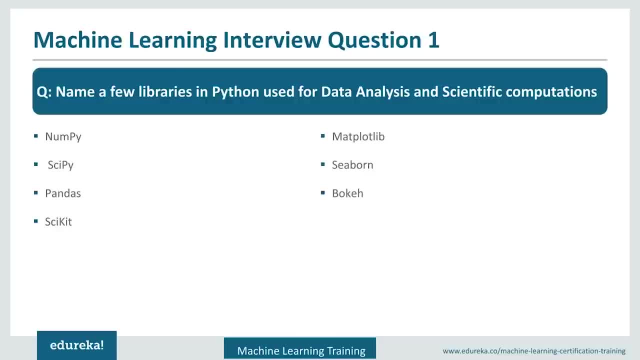 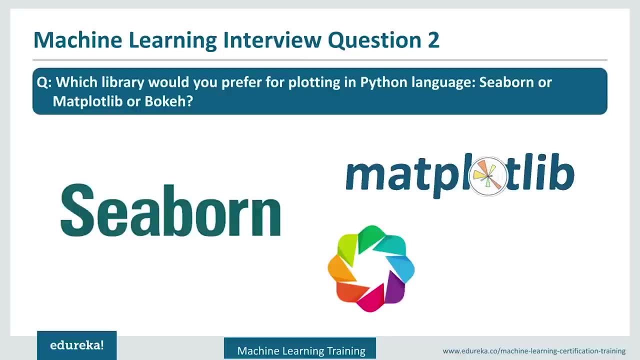 Just list them all and give a bit of a Description about the APIs and interface of their development panel in thisО each of them. so that would be enough in this case. which library would you prefer for plotting in python language? seaborn or matplotlib or bokeh? so all these three have their own applications. 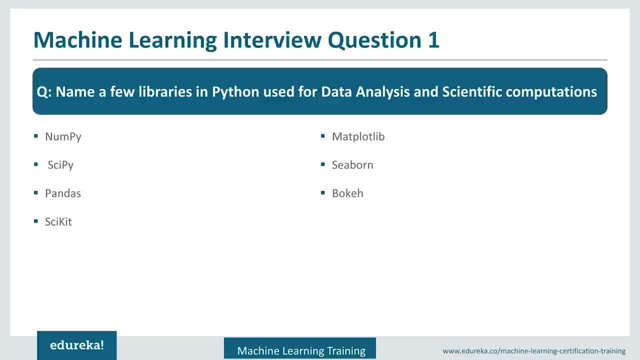 machine learning models you can use. so it contains the different components. it contains a pre-processing component where you can do the pre-processing of your data. it provides a library for that and it also provides you a different modeling library where you can access all the core machine learning models. so on top of that we have matplotlib, which is a purely of data. 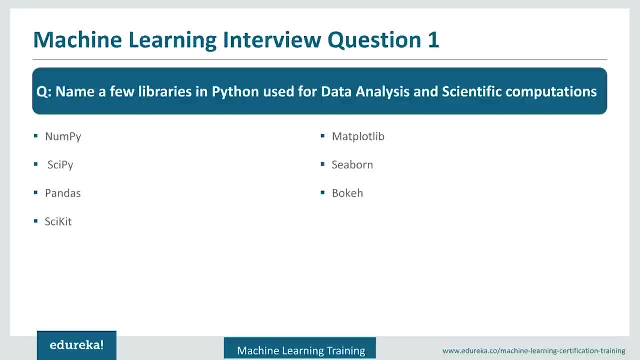 visualization tool. so with the matplotlib you can do a specific data visualization tool. so with the. So with the Matplotlib you can visualize your data in a very efficient manner and in a faster manner, And Seaborn is something which is built on top of Matplotlib. 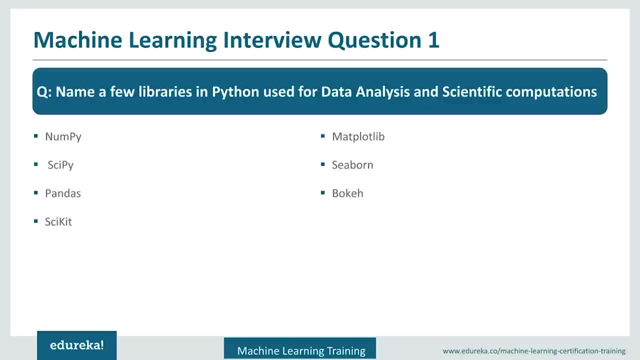 and gives you a more better visualization of the data and gives you different new kinds of visualizations which are not there within the Matplotlib. So you just can give the detail to the interviewer, just list them all and give a bit of the description about each of them. 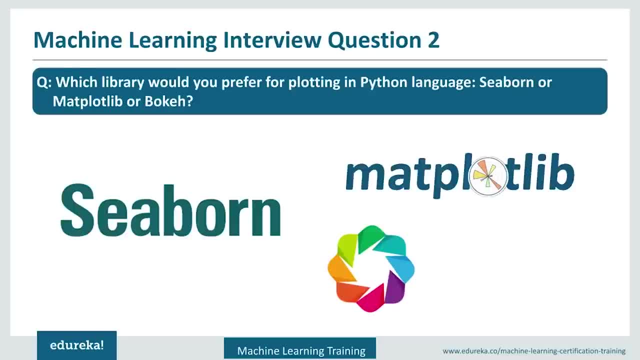 So that would be enough in this case. Which library would you prefer for plotting in Python language? Seaborn or Matplotlib or Bokeh? So all these three have their own applications. So preference is something that would come based on the thing that you're currently performing. 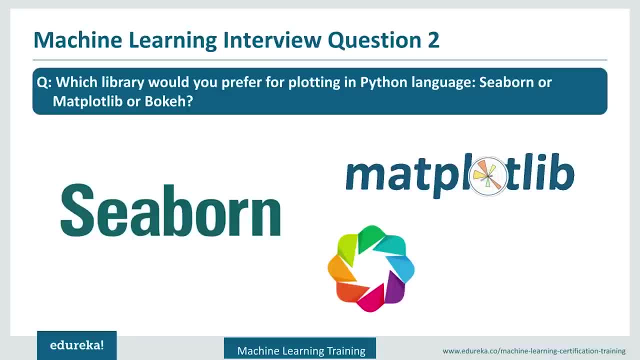 with the data analysis stage. So, for example, when you're doing a quick analysis within your data so you want to have a quick access to the charts, then you can use the Matplotlib, For example. Matplotlib provides you a quick access. 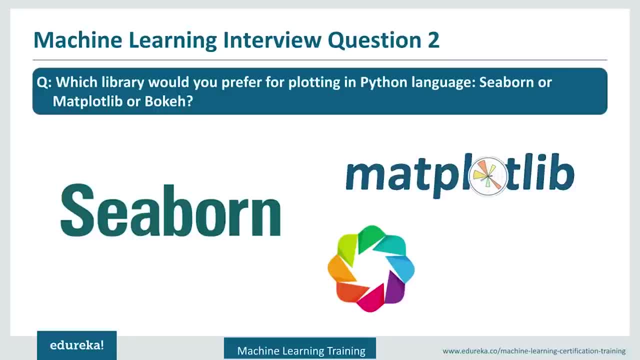 to the bar charts, pie charts, history charts and so on, Histogram line charts, scatterplot. So for the quick analysis and your data exploration, you can go with the Matplotlib. Seaborn is something which is built on top of the Matplotlib and you can use this when you want. 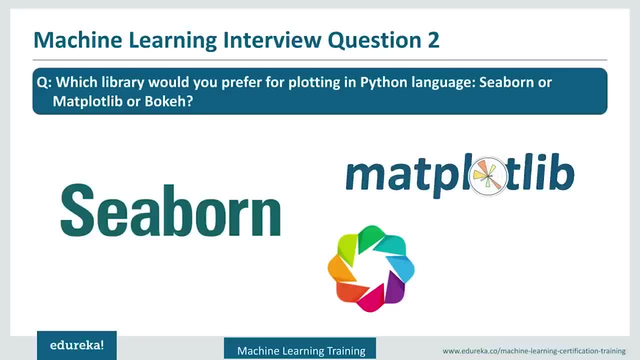 to do a bit in-depth analysis of your data, For example, when you want to have a statistical analysis within the data and Seaborn gives you a bit more types of graphs which are not there within the Matplotlib. So, for example, when you want to have a distribution. 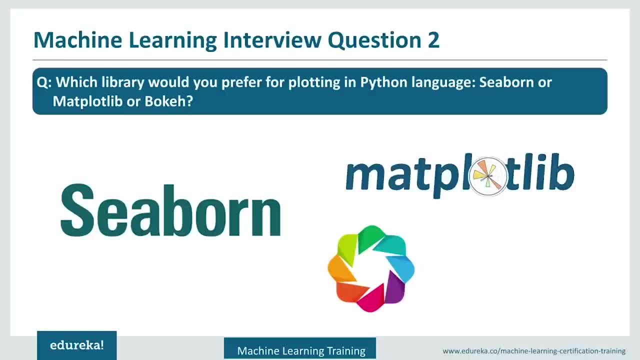 of charts with more detail. so Seaborn provides you charts such as the violin plots. it gives you a KD plots. So for the detailed explanation of your data you can go with the Seaborn. Bouquet is something which is an interactive visualization. 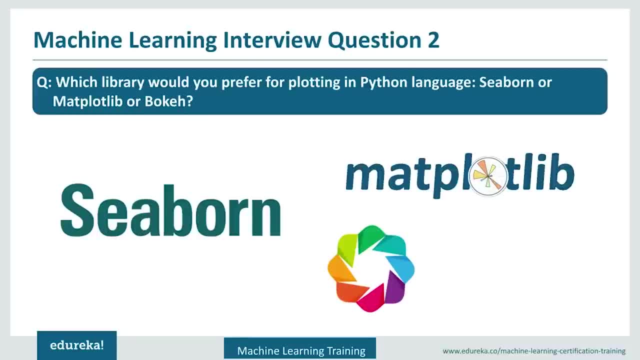 so preference is something would come based on the thing that you are currently performing with the data analysis stage. so, for example, when you're doing a quick analysis within your data so you want to have a quick access to the charts, then you can use the matplotlib, for example. 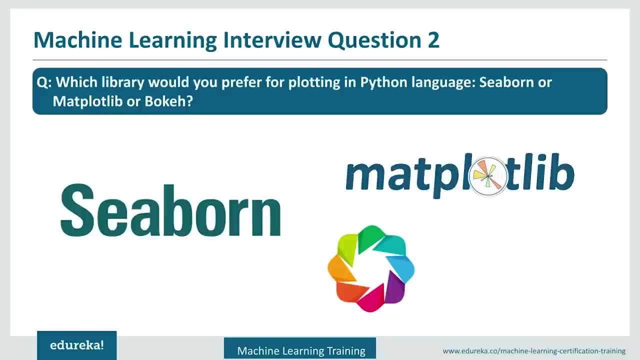 matplotlib provides you a quick access to the bar charts, pie charts, histogram line charts, scatter plot. so for the quick analysis and your data exploration, you can go with the matplotlib. seaborn is something which is built on top of the matplotlib and you can use this when you want to. 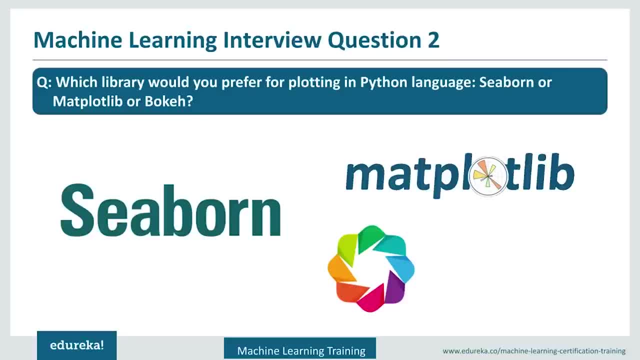 do a bit in-depth analysis of your data, for example, when you want to have a statistical analysis within the data and seaborn gives you a bit more types of graphs which are not there within the data. so you can go with the matplotlib and you can go with the matplotlib. 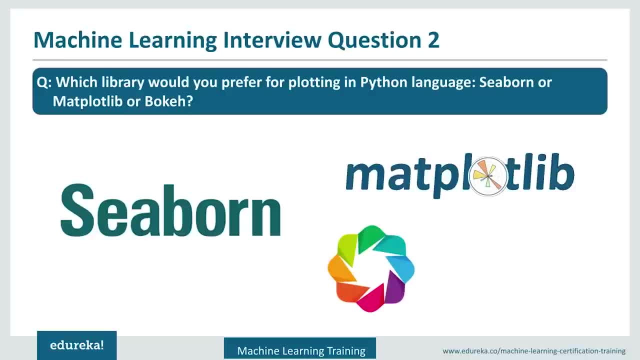 so, for example, when you want to have a distribution charts with a more detail, so seaborn provides you charts such as the violin plots. it gives you a kd plots. so for the detailed explanation of your data, you can go with the seaborn. bokeh is something which is an interactive visualization. 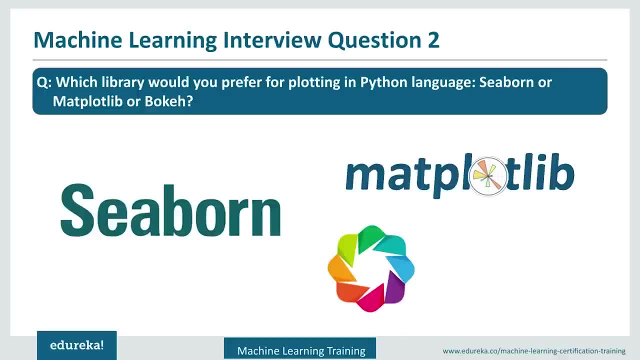 bokeh you go when you want to present your data to something of the outside world. when you want to publish it on a web and you want your user to interact with the data, then you use bokeh. so when you go to the outside and you want to publish your visualization to the outside public, 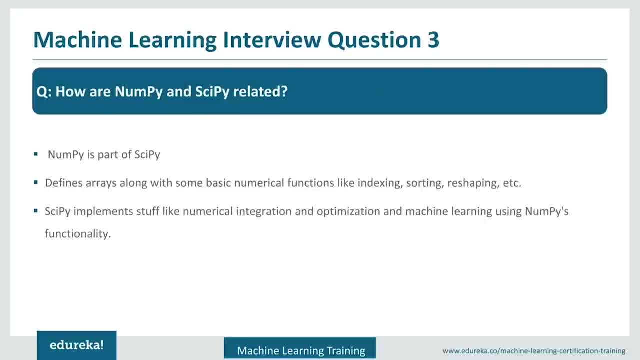 you use bokeh for that purpose. so how are numpy and scipy related to each other? so this thing, you can give a bit of detail as what is really numpy first and what is really scipy. and the thing is, scipy is a bigger library and numpy is part of it, so numpy is a smaller part of scipy. 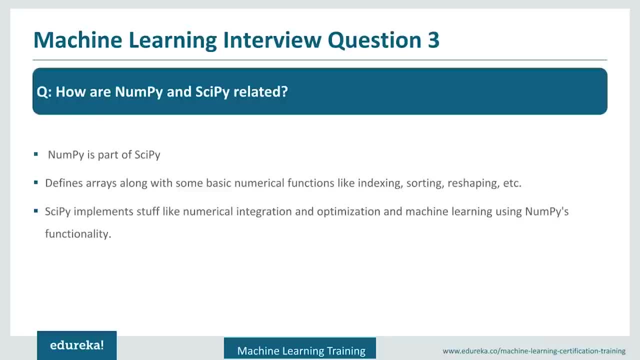 numpy helps you to define arrays and you can perform some operations on top of the libraries- arrays using the numpy libraries. so different types of operations are like indexing, sorting. you can change the shape of it, you can change the matrices, you can create a splits within your data, you can merge different arrays together. 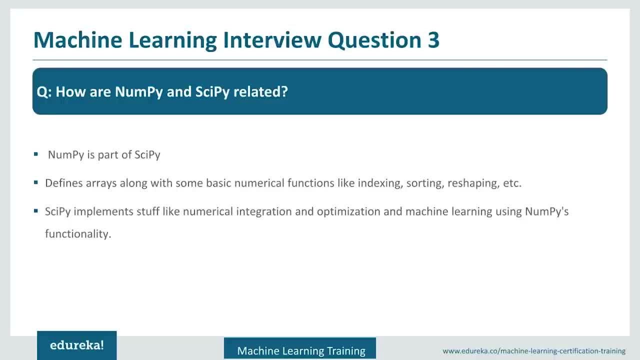 so numpy will help you with all those scipy. you can go to a next level when you using, on top of this, numpy arrays, when you want to create some mathematical formulation, you can go with this scipy. so when you want to do the optimization, you want to do the Fourier transform. if you have audio data for 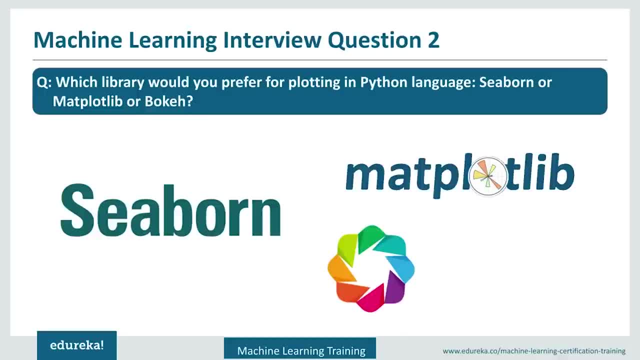 Bouquet you go when you want to present your data to something of the outside world. when you want to publish it on a web and you want your user to interact with the data, then you use Bouquet. So when you go to the outside and you want 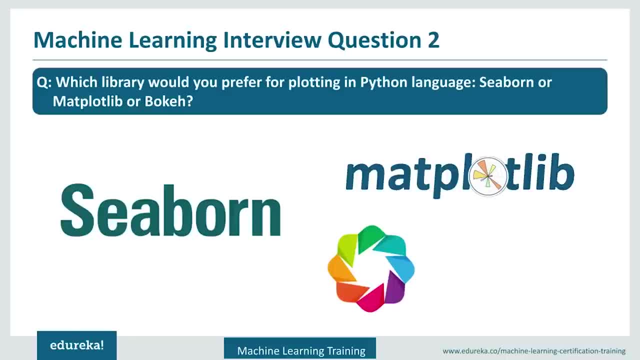 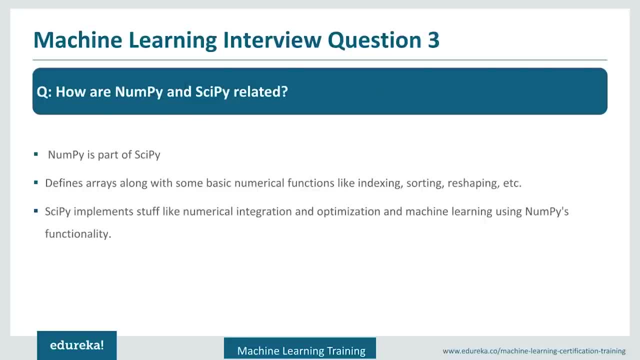 to publish your visualization to the outside world, to the outside public. you use Bouquet for that purpose. So how are NumPy and SciPy related to each other? So this thing: you can give a bit of detail of what is really NumPy first and what is really SciPy. 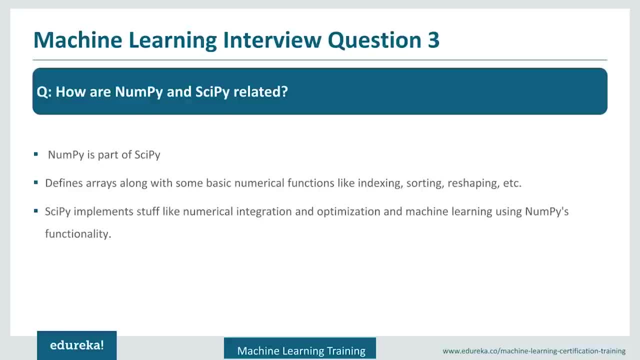 And the thing is, SciPy is a bigger library and NumPy is part of it, So NumPy is a smaller part of SciPy. NumPy helps you to define arrays and you can perform some operations on top of those arrays using the NumPy libraries. 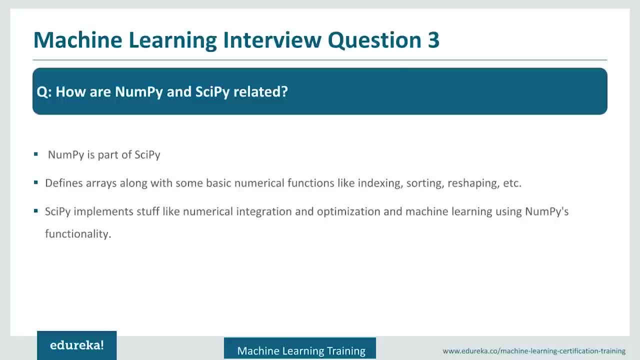 So different types of operations are like indexing, sorting. You can change the shape of it, You can change the matrices, You can create a split within your data, You can merge different arrays together. So NumPy will help you with all those. 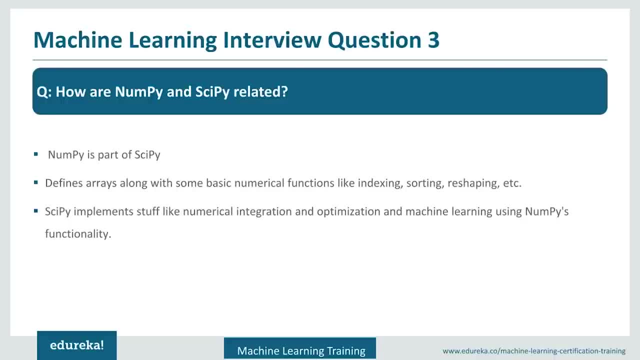 SciPy, you can go to a next level when you're using on top of those NumPy arrays. when you want to create some mathematical formulation, You can go with the SciPy. So when you want to do the optimization, you want to do the Fourier transform. 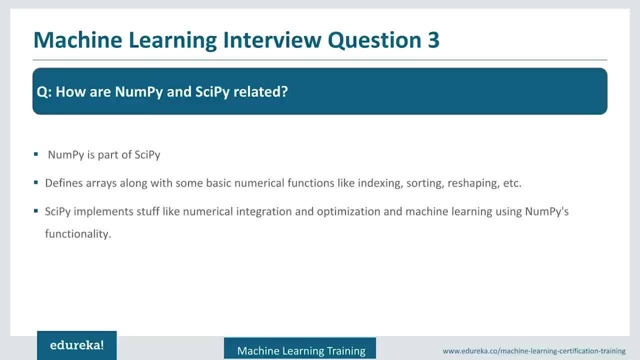 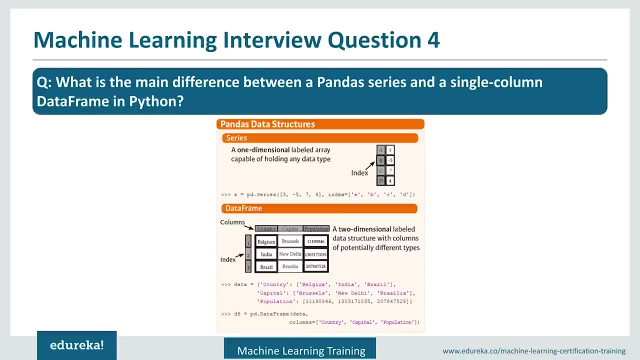 If you have audio data for those kind of applications, you can go with the SciPy. So what is the main difference between a Panda series and a single column data frame in Python? So, interviewer, he would like to really understand if you know the core concepts within the Python or not. 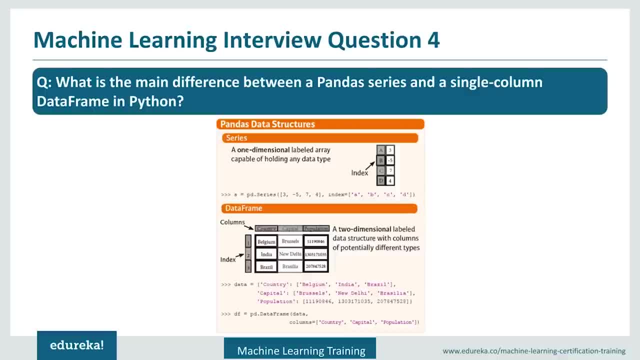 Pandas is something which is the core of the data analysis, as all your data is stored within Pandas and you're dealing with Pandas most of the time. So in this case, interviewer will try to gauge you, as you know, the basic terms which are there within the Pandas or not. 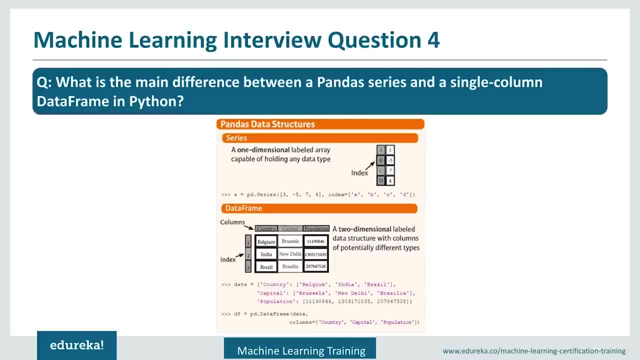 So, first thing, data frame is something which can store multiple columns, but a series cannot store multiple columns. So series is just a single column, but with the data frame, even if it's a single column, you can go with the multiple columns. 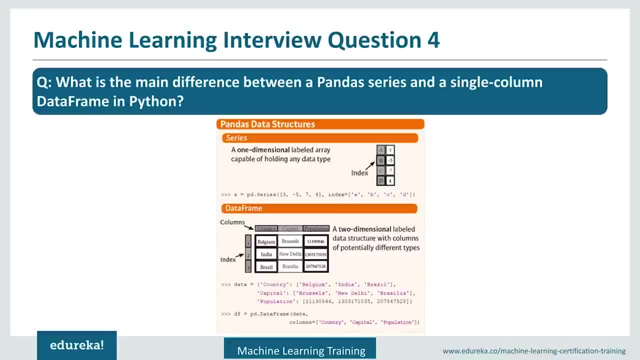 those kind of applications, you can go with the scipy. so what is the main difference between a panda series and a single column data frame in Python? so, interviewer, he would like to really understand if you know the core concepts within the Python or not. and pandas is something which is the core of the data. 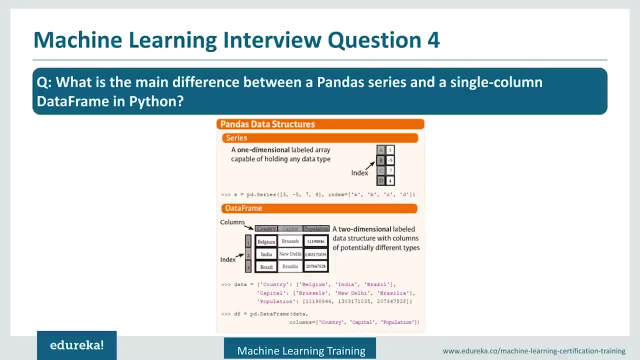 analysis, as all your data is stored within pandas and you are dealing with pandas most of the time. so in this case, interview- we try to go as you. as you know, the basic terms which are there within the pandas are not so. first thing, data frame is something which can store multiple columns, but a 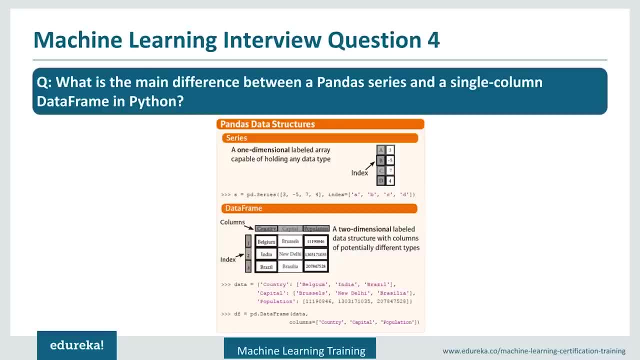 series cannot store multiple columns, so series is just a single column but with the data frame, even if it's a single column, you can go with the multiple columns, you can add the columns to it and there are some limited functions which are there with the series and data frame has additional functions on top of. 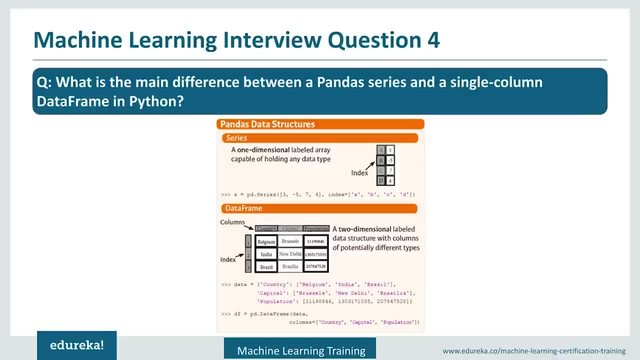 series. so, for example, LOC is a function which is there on top of this. so data frame is the upper level layer on top of series and gives you more control to the data. but the basic difference is with the series you just have a single column, but with the data frame you still can add more columns to. 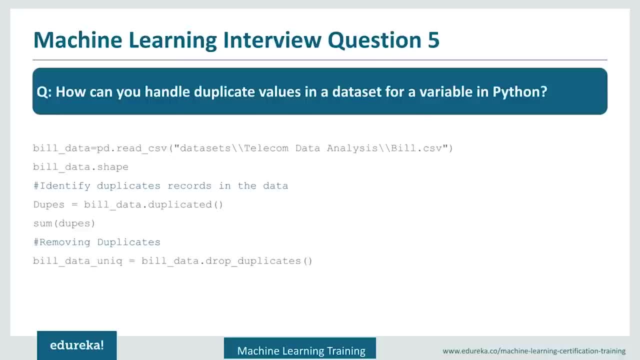 the data. how can you handle duplicate values in data set for a variable in Python? so in this case you may have to write a code and show to the interviewer that how you can really achieve this thing so you can just import the pandas library. show that you are just reading a random. 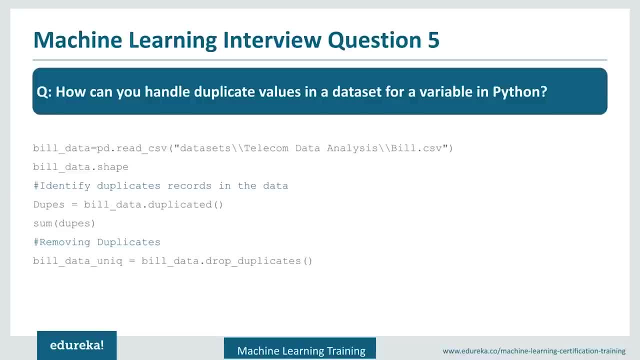 using the PD dot read underscore CSV and you use the bill data framed or duplicated to get the list of all the duplicate values which are there within the data and just show that you can also drop those columns. if sometimes we want to drop those, they are by some mistake created by the collector, so the 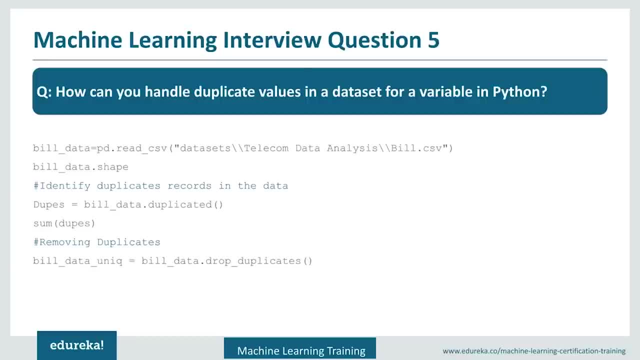 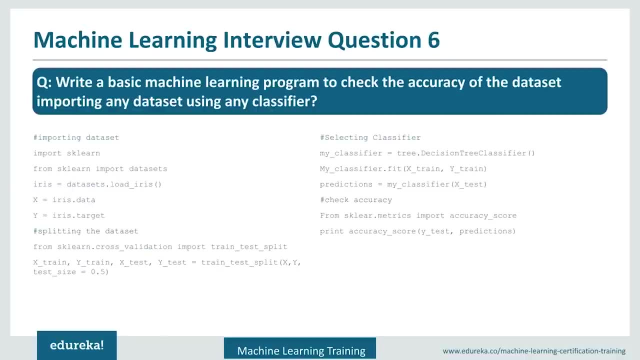 duplicate values can be removed using the drop under code duplicate columns. so these two functions. you can try to show and explain them what they do. that would help you in that. write a basic machine learning program to check the data frame and the duplicate values. you can try to show and explain them what they do. that would help you in that. write a basic machine learning program to check. 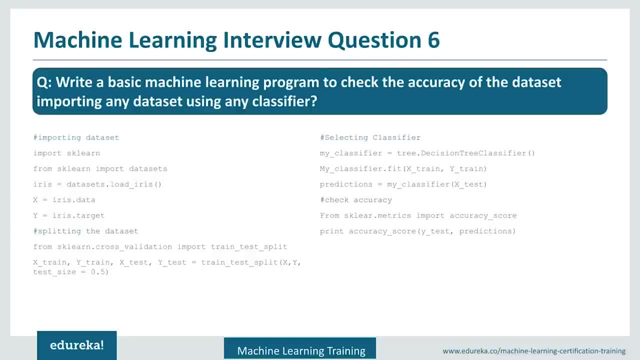 the accuracy of the data set, importing any data set using any classifier. so in this case, you're not limited with what data set you are loading water to classify. the important thing which we have to show is how you are loading your performance parameters and things that the interview will. God is how you are. 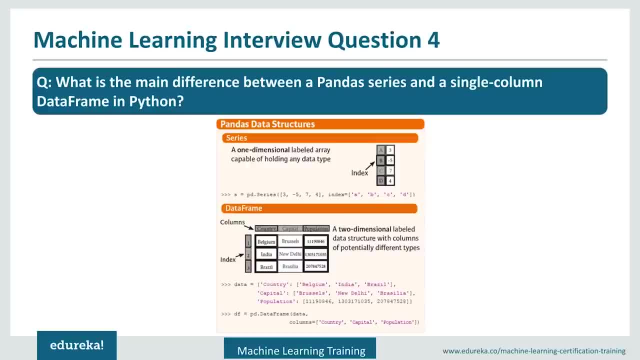 you can add the columns to it And there are some limited functions which are there with the series and data frame has additional functions on top of series. So, for example, LOC is a function which is there on top of this. So data frame is the upper level layer on top of series. 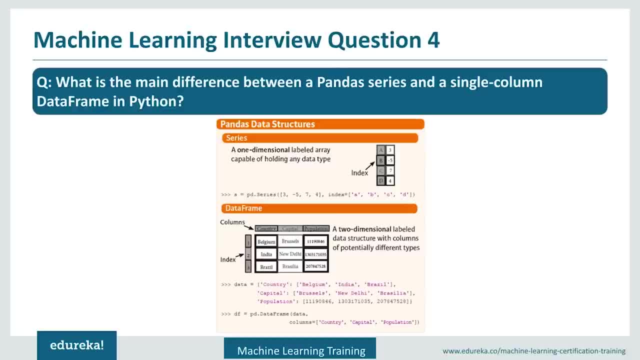 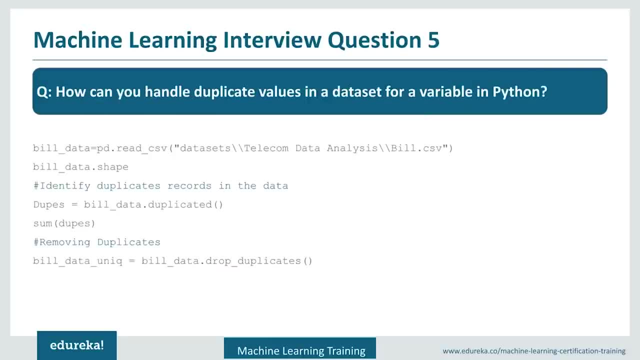 and gives you more control to the data. But the basic difference is with the series you just have a single column, but with the data frame you still can add more columns to the data. How can you handle duplicate values in dataset for a variable in Python? 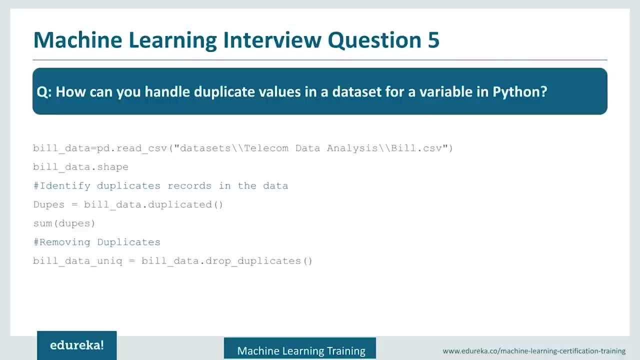 So in this case you may have to write a code and show to the interviewer that how you can really achieve this thing. So you can just import the Pandas library. show that you're just reading a random file using the pdread underscore csv. 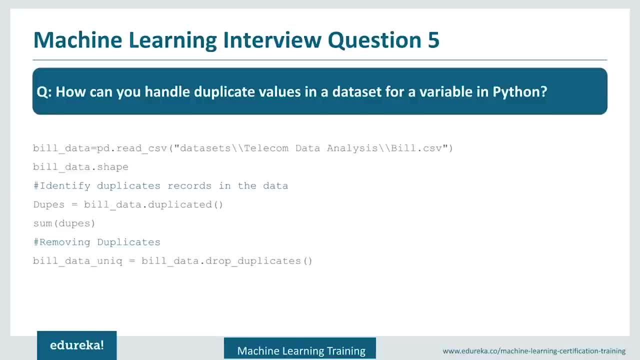 and you use the build data frame dot duplicated to get the list of all the duplicators. So you can just show that you can also drop those columns. if sometimes we want to drop those, They are by some mistake created by the collector, So the duplicate values can be removed. 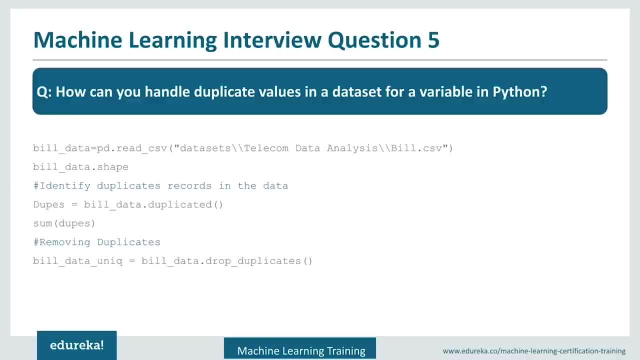 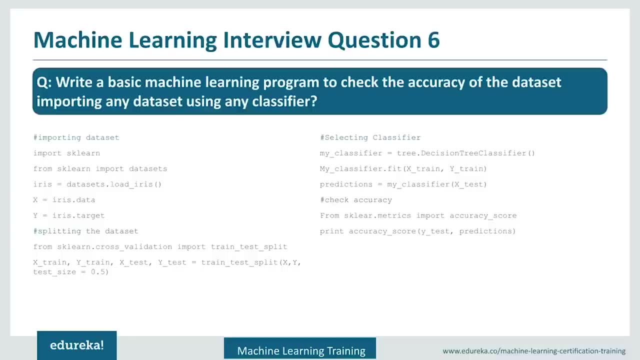 using the drop underscore duplicate columns. So these two functions. you can try to show and explain them what they do. That would help you in that. Write a basic machine learning program to check the accuracy of the dataset, importing any dataset using any classifier. 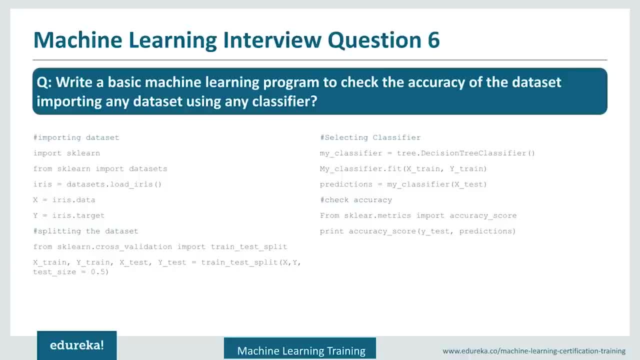 So in this case, you have limited with what dataset you are loading, what data classifier? The important thing which we have to show is how you are loading your performance parameters, and things that the interviewer will gauge is how you are trying to use the performance metrics. 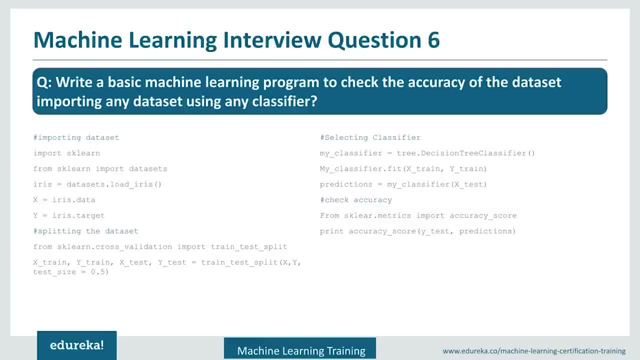 Are you trying to use it on the test set or the training set, Or you're trying to use it on the train data or just a test data? So you have to very sure you don't have the computer to do the output. you just want to write it. 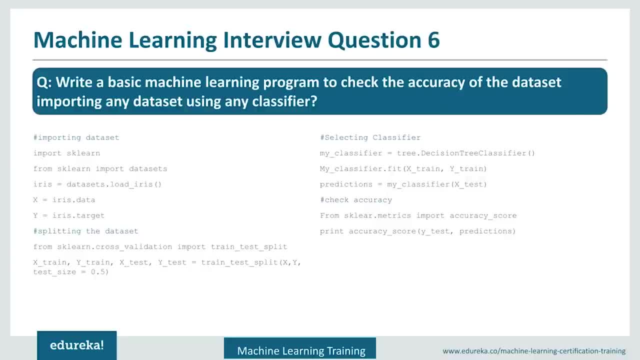 So you have to be sure that you're using it, using a test set to show the accuracy parameter, and you have to use both training y and test y in this case. so you have to start with the complete program. you have to show all the steps. 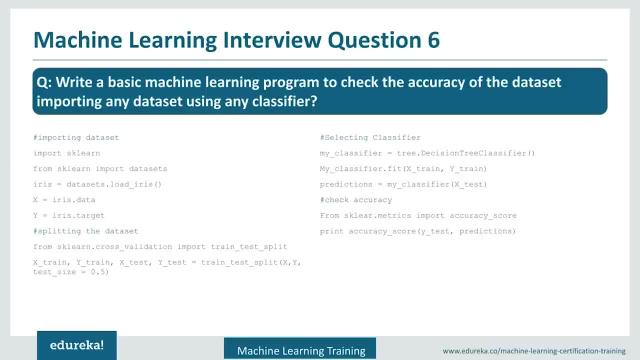 which are involved within the accuracy part. so you have to start importing your data. just take some random data- you can just show that you are reading some data- and try to separate your data into the x and y, the target data and the predictor data, and try to create a split within the data of 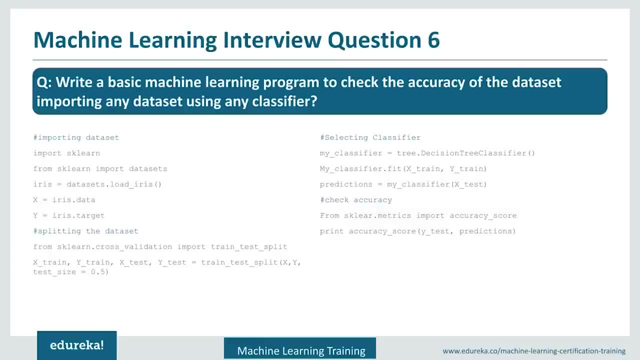 trying to use the performance metrics. are you trying to use it on the test set or the training set, or you're trying to use it on the train data or just a test data? so you have to be very sure, as you don't have the computer to do the output, you just want to. 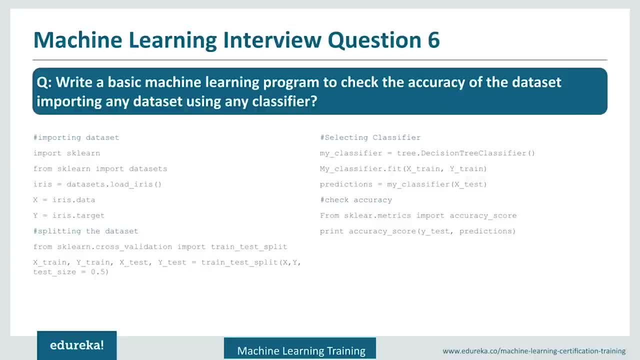 write it. so you have to be sure that you are using a test set to show the accuracy parameter, and you have to use both training y and test y in this case. so you have to start with the complete program. you have to show all the steps which are involved within the accuracy part. so you have to start. 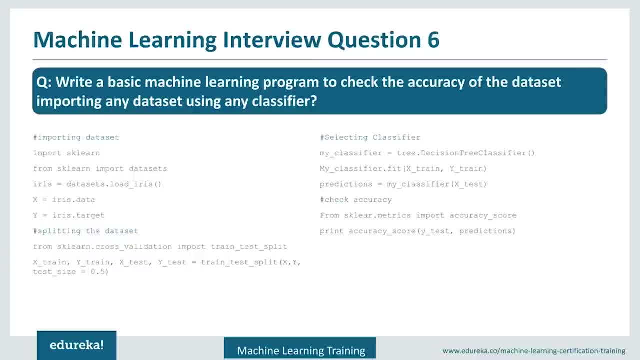 importing your data. just take some random data- you can just show that you are reading some data- and try to separate your data into the x and y, the target data and the predictor data, and try to create a split within the data of train and test validations you can use. whatever the issue you 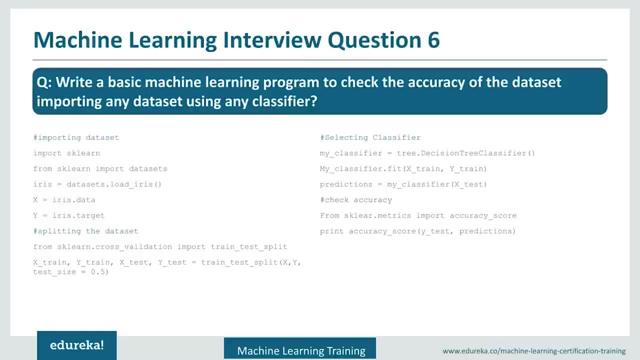 want to use. you can use 80 percent, 70 percent, 50 percent as you like, but you need to give some justification to that, also if your interviewer asks for it. once you split our data into train and test set, the next task is to use the classifiers to train the data and create a. 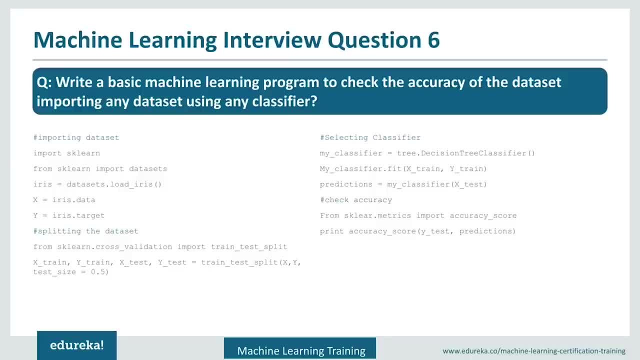 model. okay. so you can use any classifiers here, but choose something which you already know better, because interviewer will ask you whatever model you are going to use in the next step. so you have to be sure whatever you're using, you know it better. so once you have created a instance, you can use it. 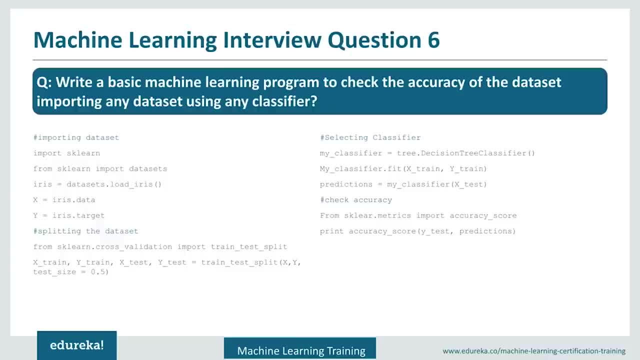 to fit it on the training data. so use the x train data and the y train data, create a model. once you have done that, you use it to make predictions on top of the test data. so you use the x test and create a predictions out of it, and accuracy tries to. 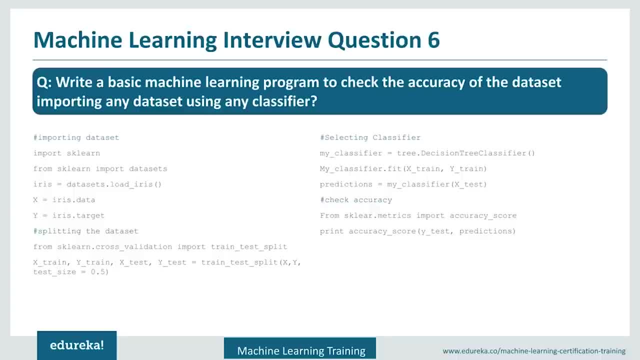 compare your data, like your original data and whatever predictions you have done, and give you a score out of it. so you will load the metric accuracy score from the sk learn matrix. once you have done that, you use the print to use the accuracy score, and accuracy score will take two. 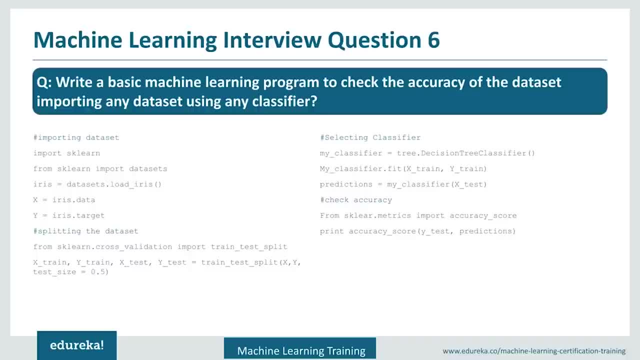 parameters. one is the original matrix, which is the y test comma, the predictions which you have currently made. so once you get that it will create a accuracy measure for that. so accuracy will be nothing but the true positive after that. so you can use the x t and x t to create a accuracy measure. 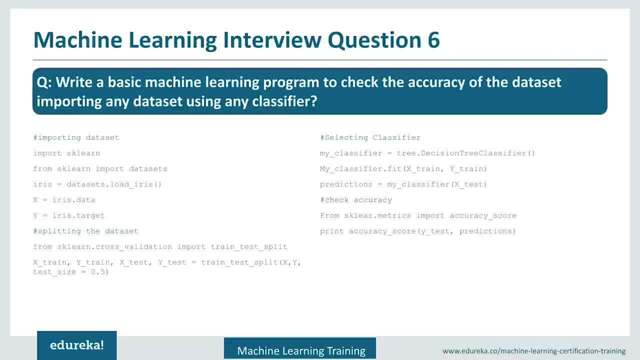 train and test validations. you can use whatever the issue you want to use. you can use 80, 70, 50 as you like, but you need to give some justification to that, also if your interviewer asks for it. once you split our data into train and test set, the next task is to use the classifiers to train. 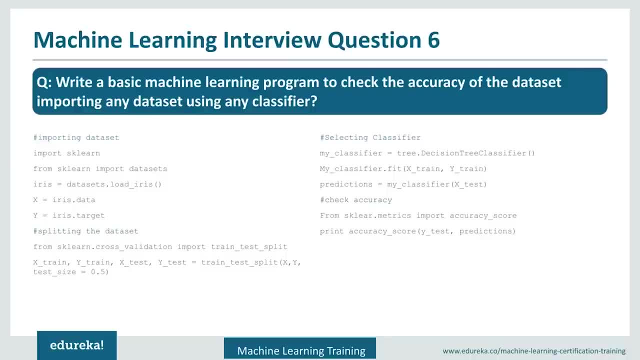 the data and create a model out of it so you can use any classifiers here. but choose something which you already know better, because interviewer will ask you whatever model you are going to use in the next step. so you have to be sure. you have to be sure what model you are going to use in the next step. so you have to be sure. 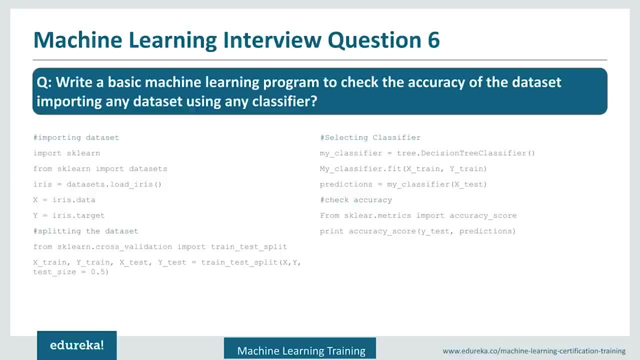 whatever you're using, you know it better. so once you have created a instance, you can use it to fit it on the training data. so use the x train data and the y train data, create a model. once you have done that, you use it to make predictions on top of the test data. so you use the x test and create. 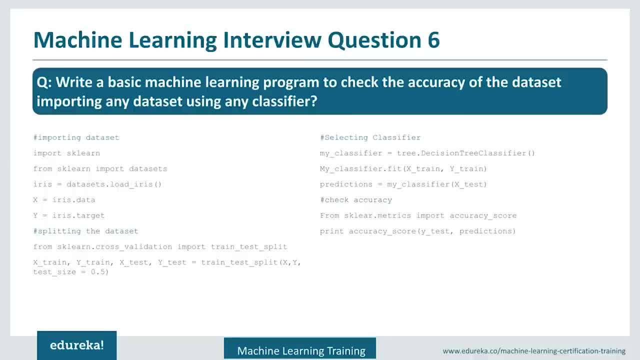 a predictions out of it and accuracy tries to compare your data, like your original data and whatever predictions you have done, and give you a score out of it. so you will load the metric accuracy score from the accuracy score and you will get a score out of it. so you will load the. 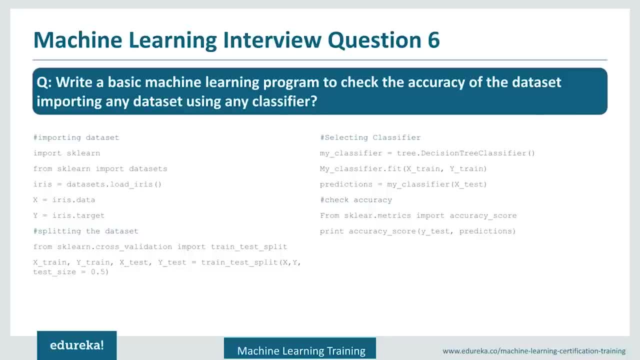 on the sk learn metrics. once you have done that, you use the print to use the accuracy score. and accuracy score will take two parameters. one is the original matrix, which is the y test comma, the predictions which you have currently made. so once you get that, it will create an accuracy measure. 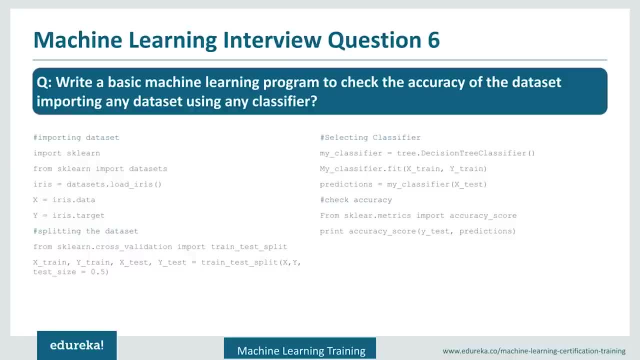 for that. so accuracy will be nothing but the true positive plus true negative upon the all data. so it will calculate that and give you. the interviewer in next step may ask you like: how can you improve the accuracy score? so once you put the accuracy score, the next thing the interview may ask you is: how can you improve? 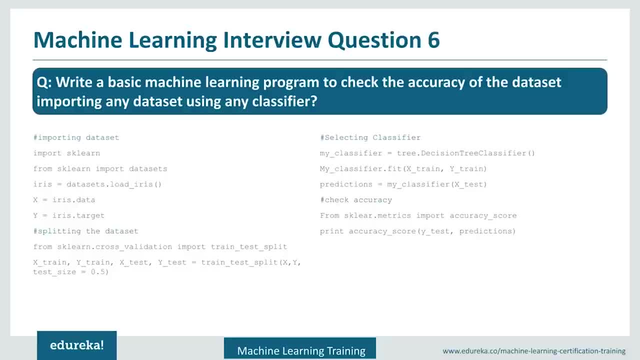 the accuracy score. so you can go for three simple steps where you can try to increase the accuracy of your model. first simple step would be: try to see if you can make some tweaking into your probability cutoff. so the default probability cutoff is 50 percent, so the ones which are above 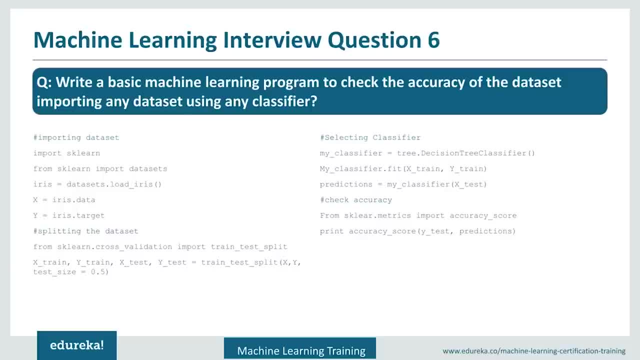 the 50 percent is tagged as one and the ones below the 50 percent probability they're tagged as zero. so changing it to something like 0.8 and then checking the accuracy: if it makes changes to your model, it is still good. if it doesn't, the next step would be try to see if you can find out some better. 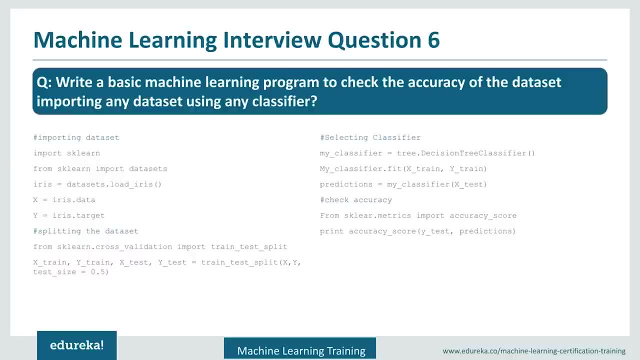 positive plus true negative upon the all data. so it will calculate that and give you. the interviewer in next step may ask you like: how can you improve the accuracy score? so once you put the accuracy score, the next thing the interviewer may ask you is: how can you improve the accuracy score? so you: 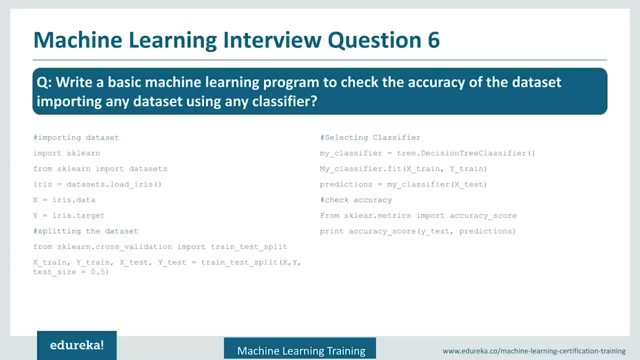 can go for three simple steps where you can try to increase the accuracy of your model. first simple step would be try to see if you can make some tweaking into your probability cutoff. so the default probability cutoff is 50, so the ones which are above the 50 is tagged as one and the 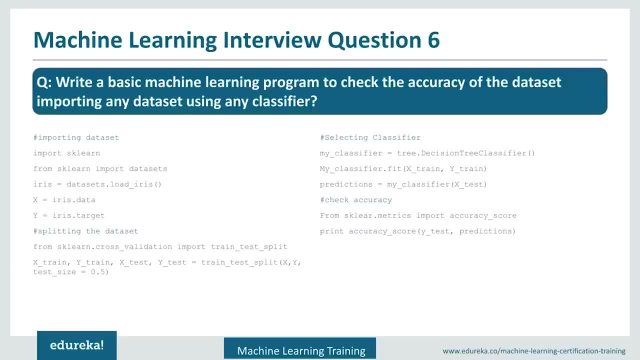 ones below the 50 probability, they're tagged as zero. so if you are changing it to something like 0.8 and then checking the accuracy, if it makes changes to your model, it is still good. if it doesn't, the next step would be try to see if you can find out some better features using some 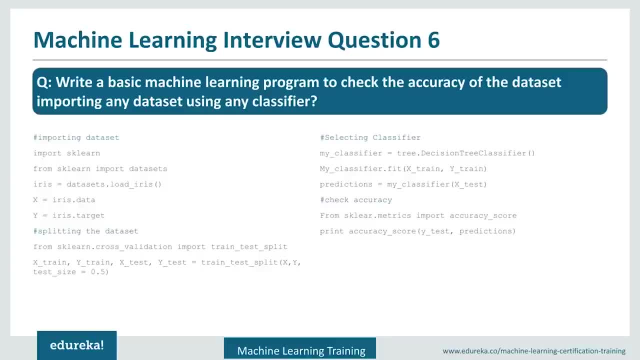 feature importance. algorithms such as random forest and different tree models are available which will give you the better features as per the target. so you can use those features and train a model so that you will have your accuracy increased. and next step would be create some new features and see if your 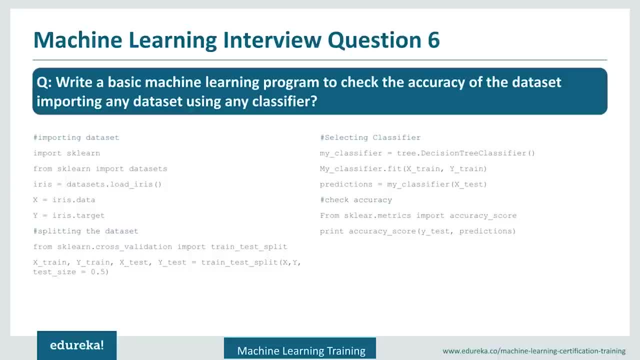 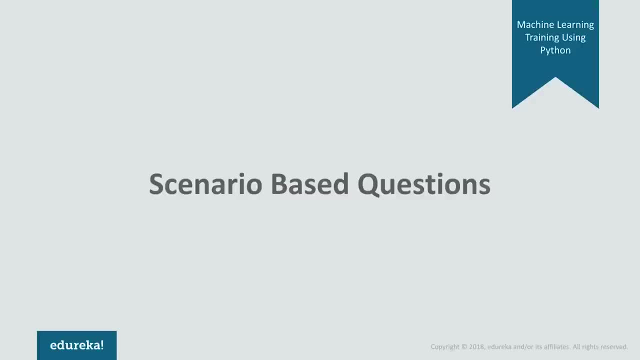 model makes any improvement in your accuracy, you can make some new features or you can add some more data so that it will help your model to generalize better. for this part, we have completed with the python related interview questions of the machine learning, so this was more of a technical. 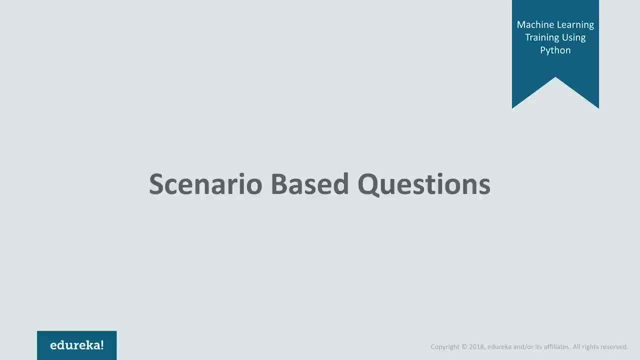 and technical part that we are going to discuss in this video. now let's move on to the scenario based questions, where we can see how you can code, how we can show the interviewer that interview is more interested to see how you can code the things and how confident you are with those things. okay, 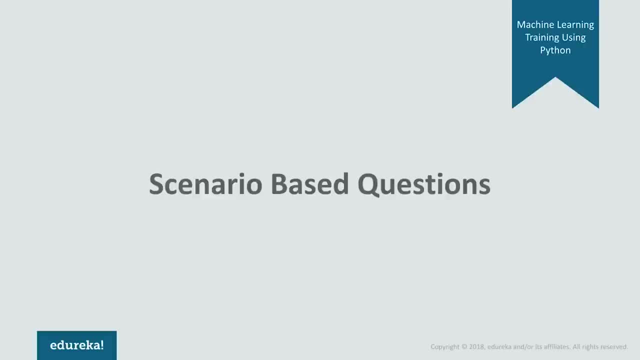 so now we are done with that, we will now move on to the scenario based questions, where we will see some puzzle kind of things, and the other are real problems where the interview is related to understand as how you try to solve those problems. let's start with those. so you are given a data set. 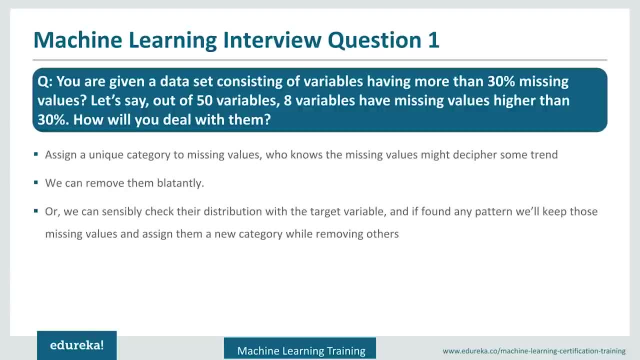 of missing values. Let's say, out of 50 variables, 8 variables are missing values higher than 30%. How will you deal with them? So missing values could be of any reasons. Something like it's: your data got corrupted while storing and you got a missing data. The person who collected the data? 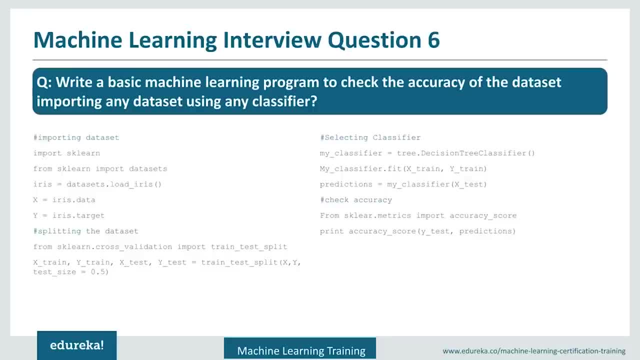 features using some feature importance. algorithms such as random forest and different tree models are available which will give you the better features as per the target. so you can use those features and train a model so that you'll have your accuracy increased and next step would be create. 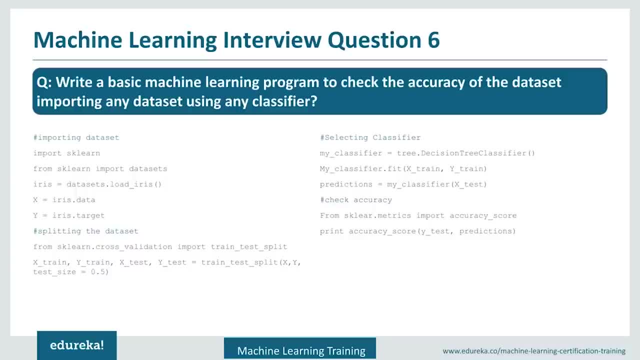 new features and see if your model makes any improvement in your accuracy. you can make some new features or you can add some more data so that it will help your model to generalize better. for this part we have completed with the python related interview. questions of the machine. 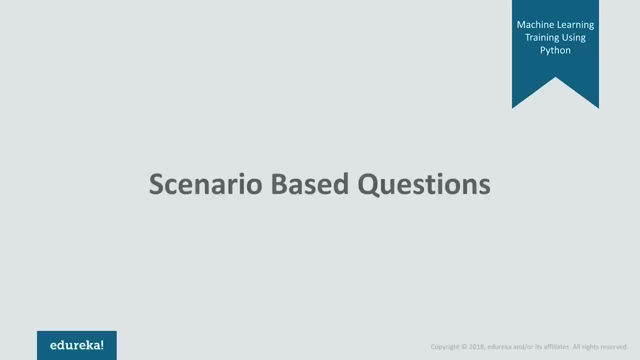 learning. so this was more of a technical part of it, where we saw how we can code, how we can show the interviewer that interview is more interested to see how you can code the things and how confident you are with those things. okay, so now we are done with that. 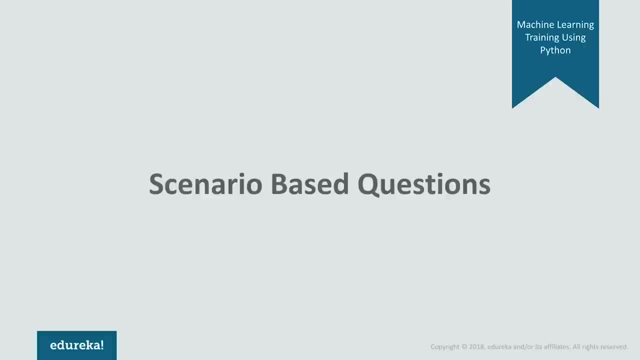 we will now move on to the scenario based questions, where we will see some puzzle kind of things and the other are real problems where the interview is related to understand as how we use. try to solve those problems. let's start with those. so you are given a data set consisting of: 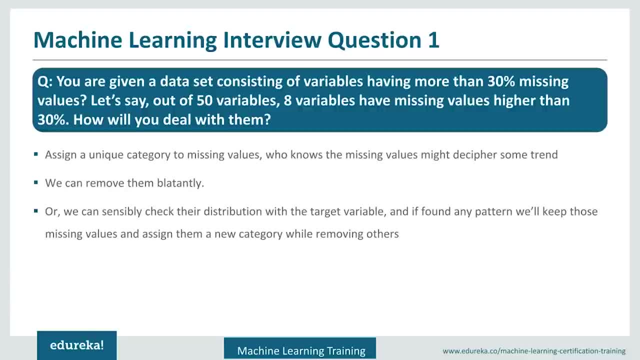 variables having more than 30 percent of missing values. let's say, out of 50 variables, eight variables are missing values higher than 30 percent. how will you deal with them? so missing values is a par of two kinds of values. you will receive one of the values which includes the. 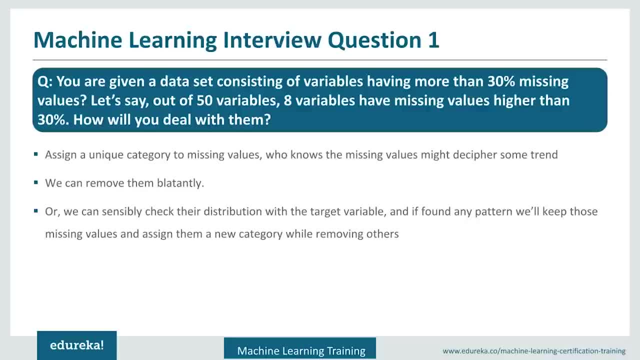 data set, meaning from any data set you clicked on the calculators function and that data you collect from that data set is your data set worth in-house. so, for example, let's say, i collected for anything know you collected from a certain variable, i collected from a certain value. so, for example, that I collected out from here, 이것 data. 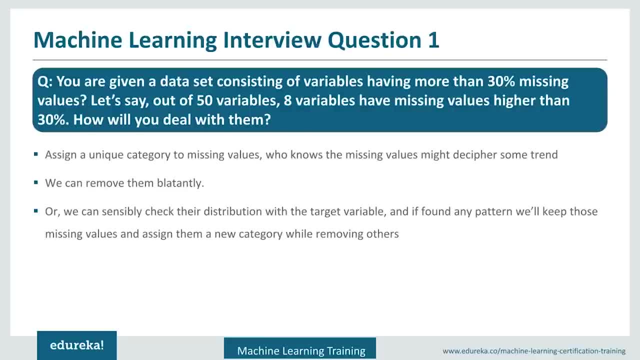 dicho una總 de capital de sitten data. i got my data listed in-house as a data set. so how will we solve this problem? okay, and in what importance- and we have a question, you can look into the context we talk about that: the pre given data set from the behavior of the data set. so 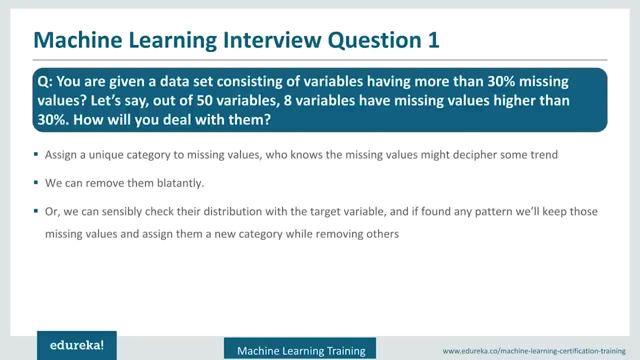 you have values like your data are not important, but some of the variables are finding that some of those values at the top of the data set- your data set the day that you have rain- non-missing, and this much of the part is missing. so we can assign it one and zero. we can create a. 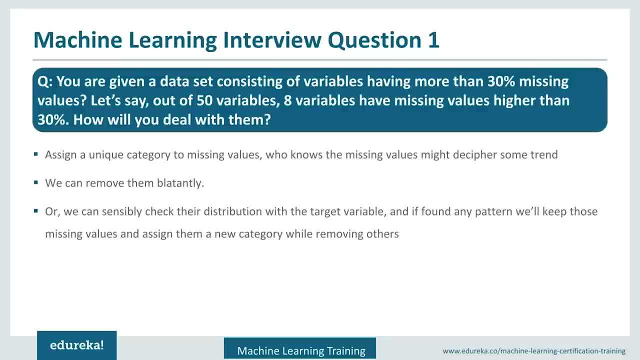 new binary variable. it's possible that this thing is trying to give you some idea about the data and there will be some hidden pattern within your data because of this, some missing values. so it's possible that creating this new feature will help your model to give the better accuracy. 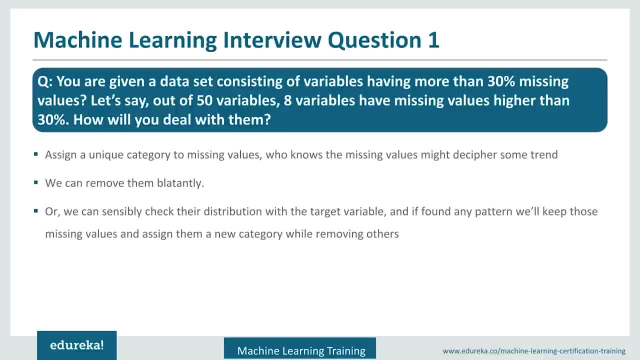 may have done some mistakes and that data is treated as a missing data, Or it could be like there is nothing for those kind of values, So it's like it is supposed to be blank and it's supposed to be missing. So there are different conditions for those. So let's see how we can try to handle. 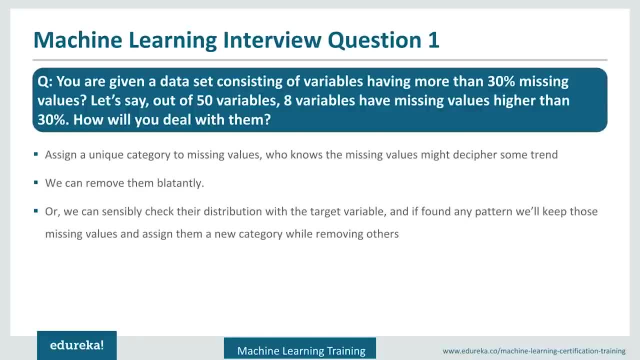 those things. First, we can create a new feature which will say: okay, this much of the part is non-missing and this much of the part is missing, So we can assign it 1 and 0. We can create a new. 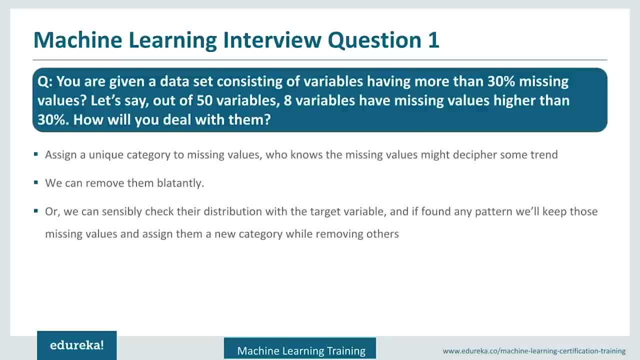 binary variable. It's possible that this thing is trying to give you some idea about the data and there will be some hidden pattern within your data because of this, some missing values. So it's possible that creating this new feature will help your model to give the better accuracy and give the better performance. Second thing we can remove: 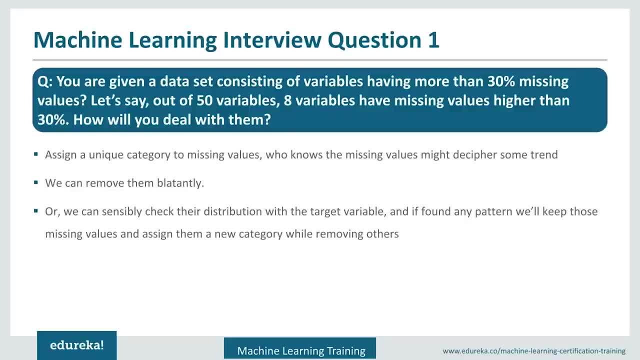 that completely if you have a high count of data. So, for example, if you have a very good amount of data and you can say that, okay, I can leave with removing this 30% of the data, then you can bluntly remove this If it is not giving any value to you and you can't spend much time on trying to. 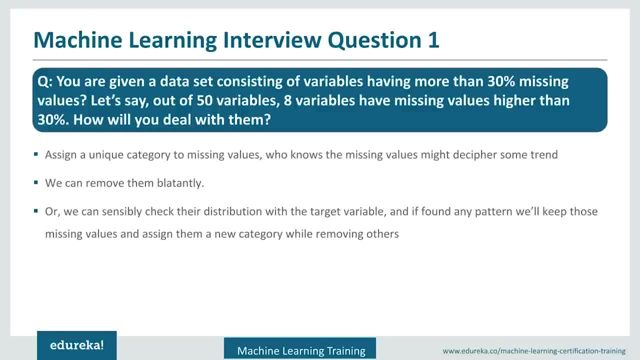 improve it or trying to impute it. then you can bluntly remove it Or you can check the distribution. For example, there are different ways to check how your missing values are to the similar clusters. So some examples are: you can see your missing values are clustered on some other values, So can 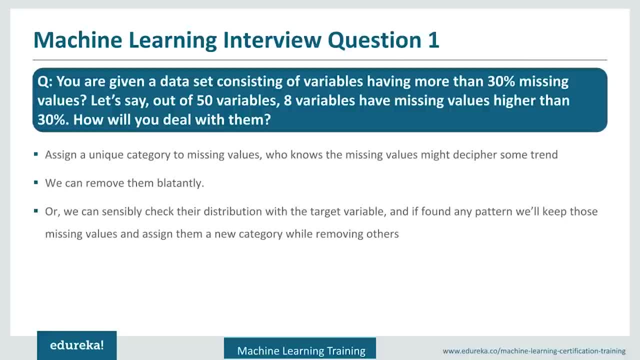 we give this cluster values to those missing values. So it's like identifying clusters and, based on those clusters, we give values to the missing data. Or the second thing is we use the distribution. So if they're continuous in nature, we can use the distribution to assign some data to. 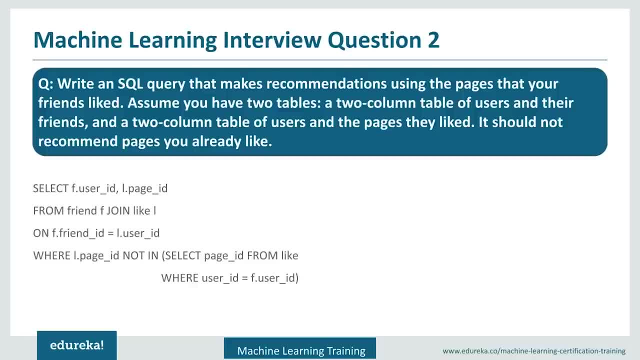 them. For example, let's say we have a table of users and their friends using pages that your friends like. So assume you have two tables. First table is a column table of users and their friends. Second table is a column two column table of users and the pages they like. It should not recommend pages you. 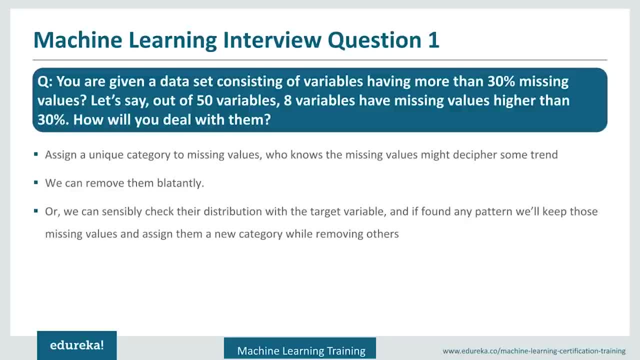 and give the better performance. second thing: we can remove that completely if you have a high count of data. so, for example, if you have a very good amount of data and you can say that, okay, i can leave with removing this 30 percent of the data, then you can bluntly remove this if it is. 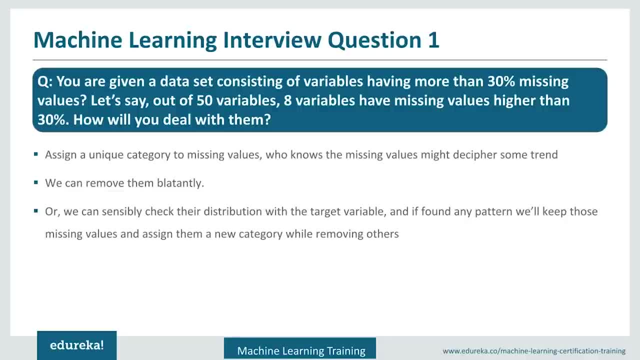 not giving any value to you and you can't spend much time on trying to improve it or trying to impute it. then you can bluntly remove it or you can check the distribution. so, for example, there are different ways to check how your missing values are to the similar cluster. so some examples are: 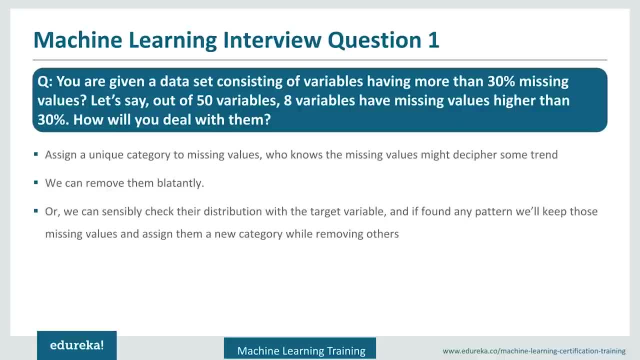 you can see your missing values are clustered on some other values. so can we give this cluster values to those missing values? so it's like identifying clusters and based on those clusters we give values to the missing data. or the second thing is we use this distribution so if they are continuous, 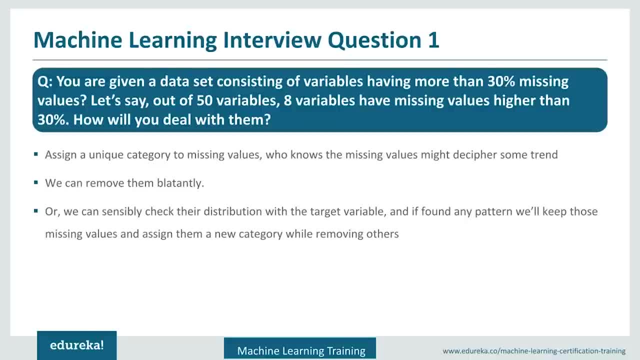 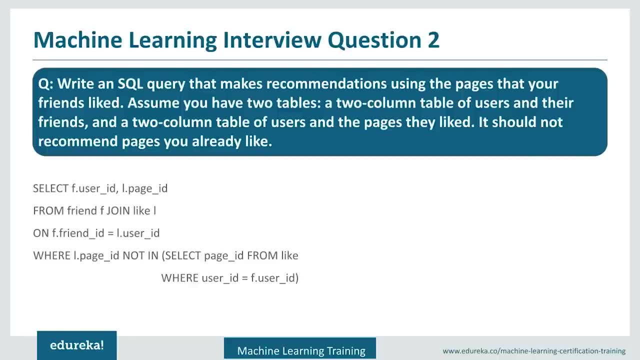 in nature, we can use the distribution to assign some data to them. so write an sql query that makes recommendations using pages that your friends like. so assume you have two tables. first table is a column table of users and their friends. second table is a column two column table of users and the pages they like it. 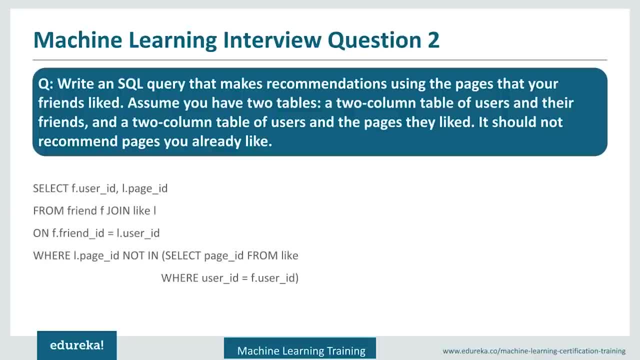 should not recommend pages you already like. so why would interviewer ask an sql question in this case? so it is like he is trying to understand how better you know the recommendation in this from the database point of view. so it is like he is trying to understand your knowledge in a different. 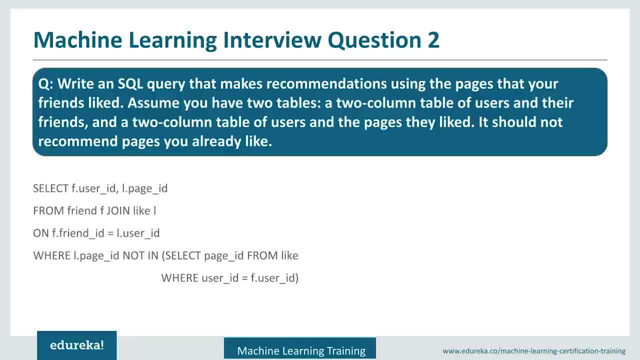 term. so first thing, you have these two tables. so first table is including- you can assume you have to make some assumptions and draw the picture of this two tables first. so first table will include a user id and a friend id. second table will include a user id, the page id they have liked, and then 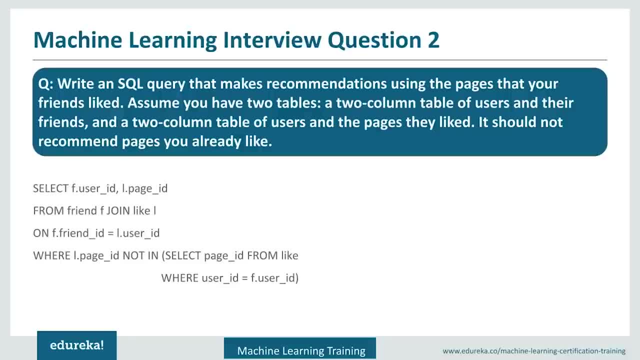 once you have this structure of these two tables ready, the next step is to merge them together based on the friends. so, as we are interested to know as which friends are liking which pages and based on that, we want to recommend it to the original user. so first thing is we have to combine these two tables using a unique key which is the friend's. 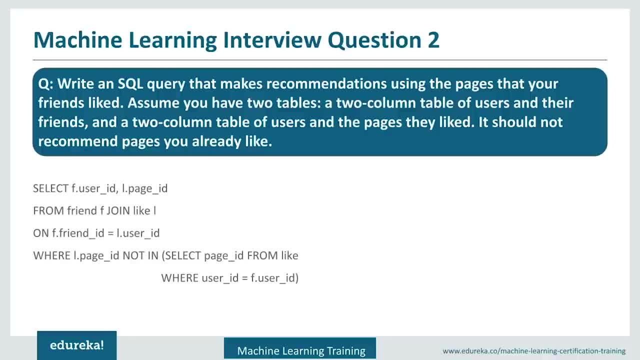 already like. So why would interviewer ask an SQL question in this case? So it is like he's trying to understand how better you know the recommendation in this from the database point of view. So it is like he's trying to understand your knowledge in a different term. So, first thing, you have this: two tables. So first table is including you can assume you have to make some. 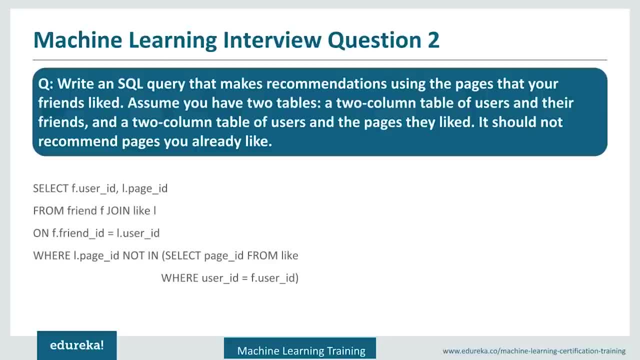 assumptions and draw the picture of this. two tables first. So first table will include a user ID and a friend ID. Second table will include a user ID, the page ID they have liked, And then, once you have this structure of this two tables ready, the next step is to merge them together based on the friends. So, as we are, 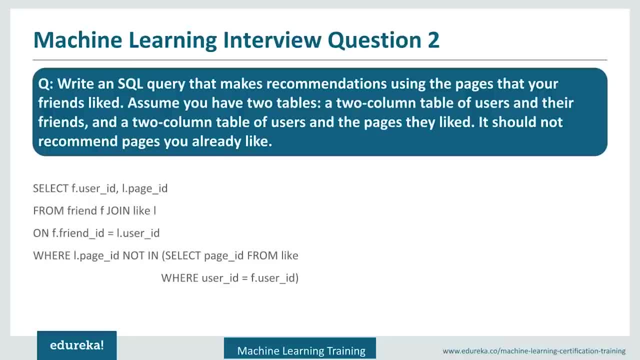 interested to know as which friends are liking which pages and based on that, we want to recommend it to the original user. So first thing is we have to combine these two tables using a unique key, which is the friends ID. So we join these two in the SQL. 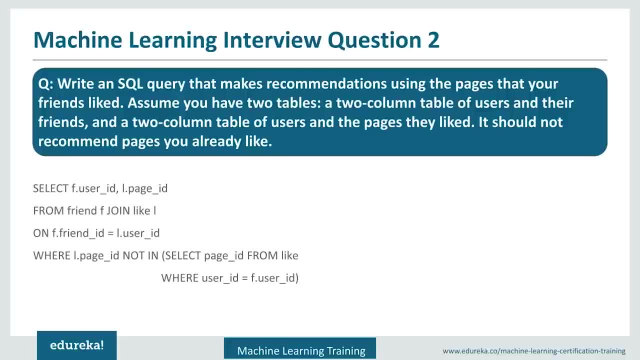 using the friends ID. That is one condition. Second condition says it should not recommend pages you already like. So what you do, you have to have a way where you can exclude the pages which were already liked by that user. So this can be done by an inner. 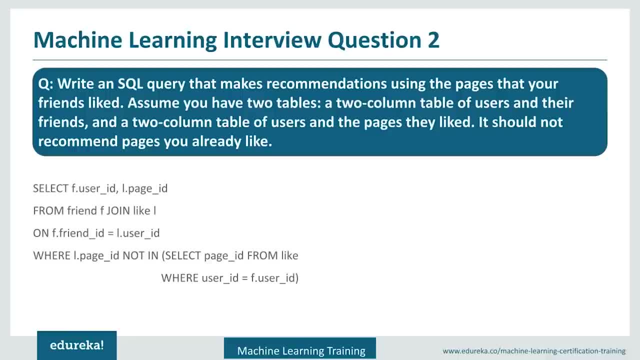 query which you can use here to select the pages which that user has already selected And in the where condition you can say: the page should not include this. So if you look at the whole query again, we are first selecting the first table: user ID. 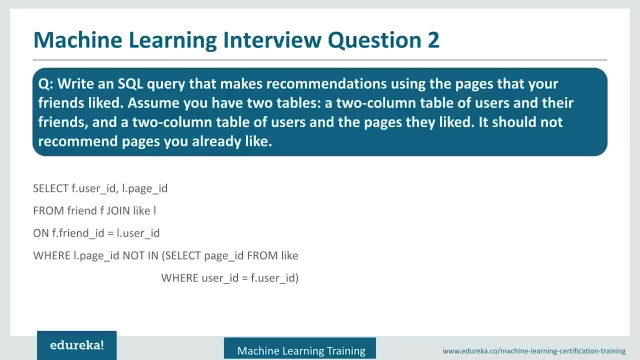 the friends table user ID and the likes table page ID from friends f join like l. So we are trying to join them together on friend ID and the user ID. Second is, as we mentioned, that was the first thing and the second thing is we try to remove the recommendations. 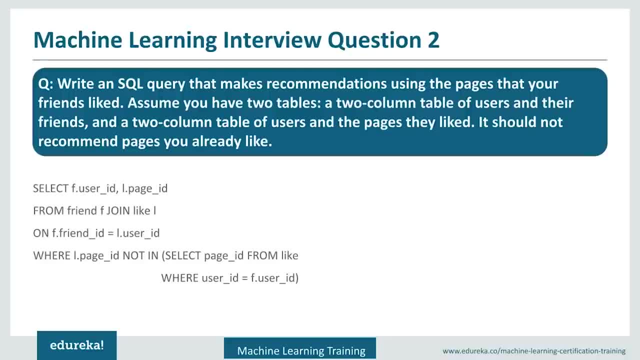 to the pages which he has already liked. So which we will do by page ID, not in the pages which he has already liked. So this is the condition which is trying to do this, and this is how you can explain this thing to the interviewer. 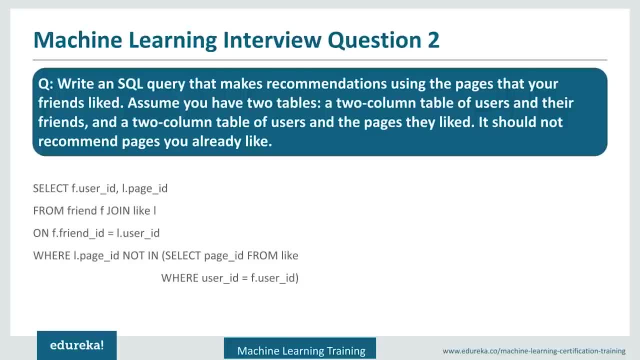 id, so we join with the sql using the friends id. that is one condition. second condition says it should not recommend pages you already like. so what you do, you have to have a way where you can exclude the pages which were already liked by that user. so this can be done by an inner query. 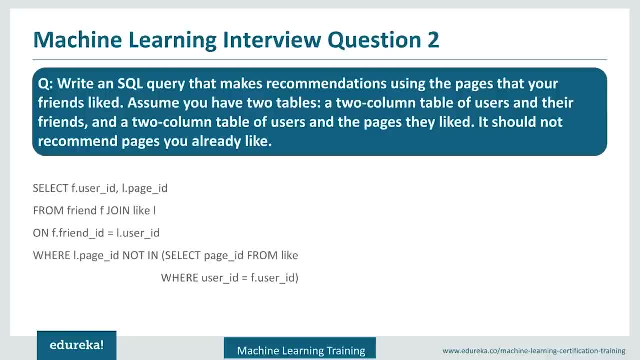 which you can use here to select the pages which that user has already selected and in the where condition you can say: the page should not include this. so if you look at the whole query again, we are first selecting the first table user id, the friends table user id and the 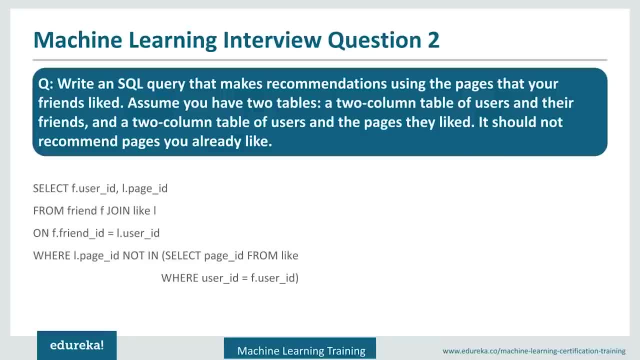 likes table page id from friends f join like l. so we are trying to join them together on friend id and the user id. second is, as we mentioned, that was the first thing and the second thing is we try to remove the recommendations, the pages which he has already liked, so which will do by page id, not in. 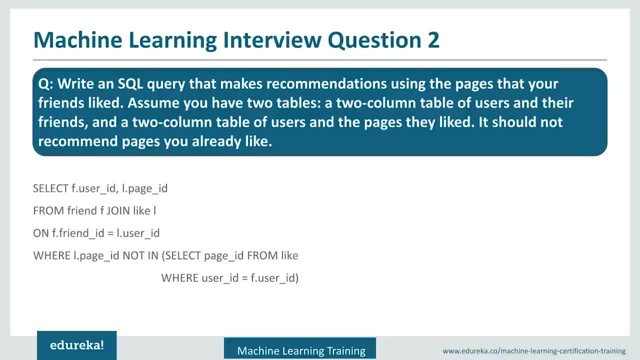 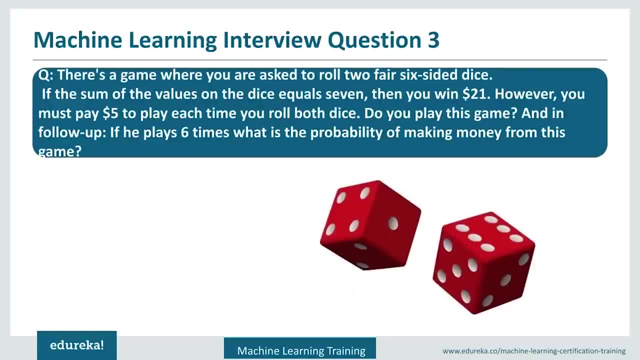 the pages which he has already liked. so this is the condition which is trying to do this and this is how you can explain this thing to the interviewer. so there is a game where you are asked to roll two fair, six-sided dice. if the sum of the values on the dice equals seven, then you 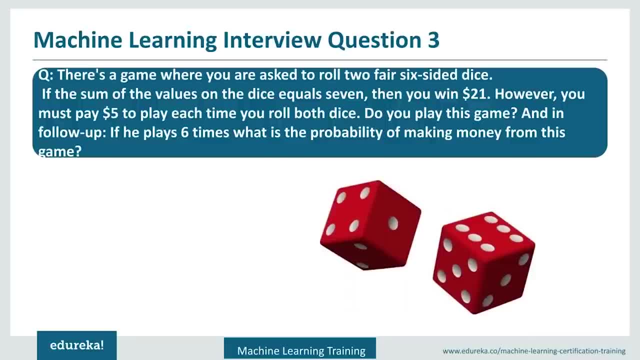 win twenty one dollar. however, you must pay five dollar to play. each time you roll both dice do you play this game? and, in follow-up, what is the probability of making money from this game if you're playing it for six times? so the first condition says: if the sum of the values on the 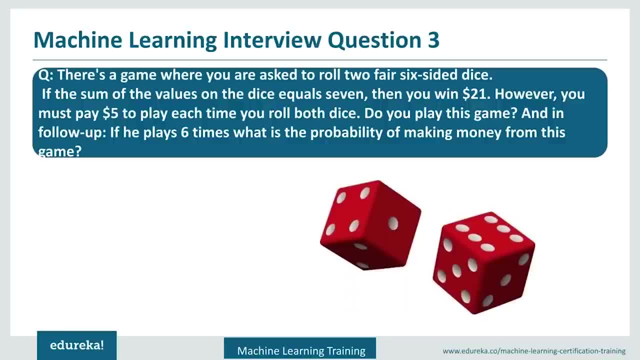 dice equals seven, then you win twenty one dollars, but for all other cases you have to pay five dollar. so in this case, if we first assume all the possible cases- as we have fair six-sided dice and we have two of them, so there is six multiplied by six, we have 36 different cases, and out of it, 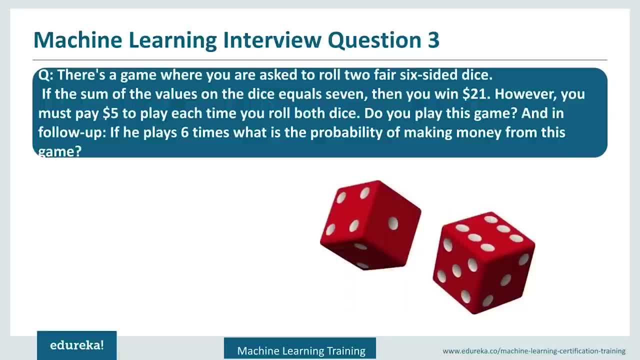 having two dices equal to seven is like we have one and six, we have two and five, we have three and four, we have four and three, we have five and two and we have one and six again. so those are nothing but six possible chances are there out of thirty six. if we take a ratio, six by thirty six will give. 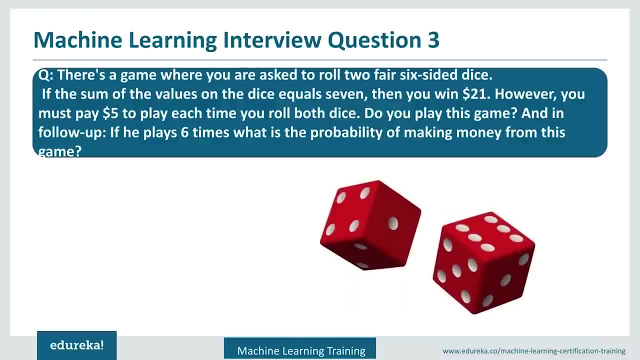 So there is a game where you are asked to roll two fair, six sided dice. If the sum of the values on the dice equals 7, then you win $21.. However, you must pay $5 to play each time you roll both dice. 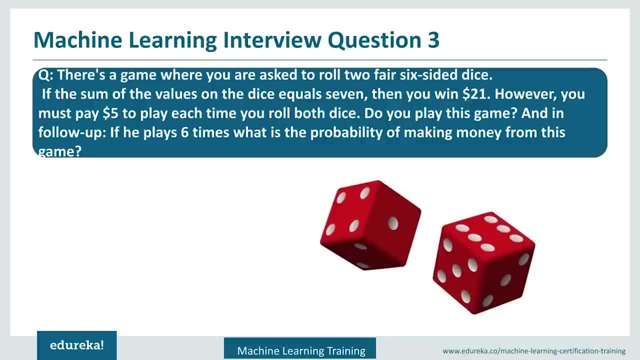 Do you play this game and, in follow up, what is the probability of making money from this game if you are playing it for six times? So the first condition says: if the sum of the values on the dice equals 7, then you win $21.. 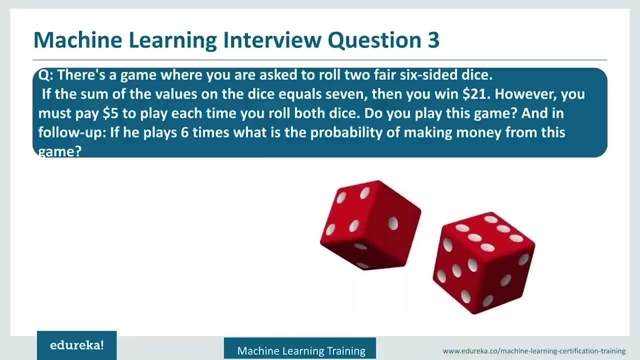 But for all other cases you have to pay $5.. So in this case, if we first assume all the possible cases, as we have fair six sided dice and we have two of them, So there is six multiplied by six, we have 36 different cases. 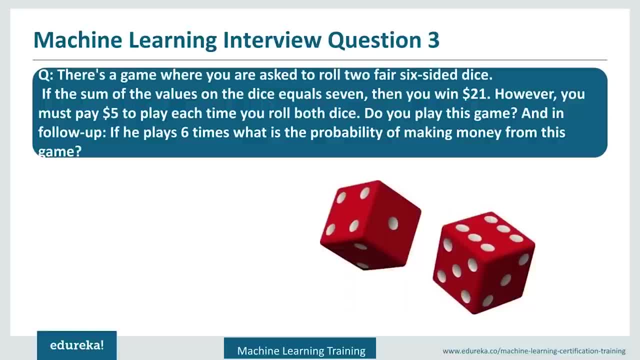 and out of it having two dices equal to seven is like we have one and six, we have two and five, we have three and four, we have four and three, we have five and two and we have one and six again. So those are nothing but six. possible chances are there. 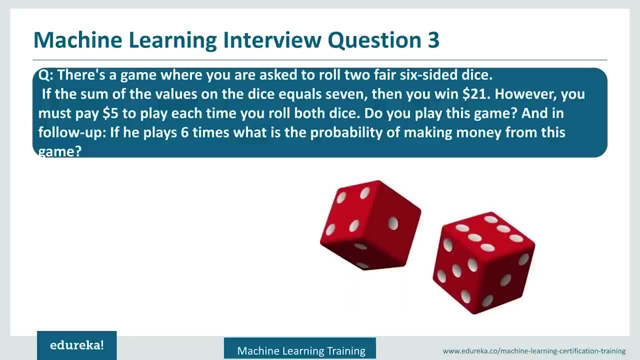 out of 36.. If we take a ratio, 6 by 36 will give us 1 by 6 ratio. So this says we have a chance of winning $21, one in six games. So assume that we are playing six games and out. 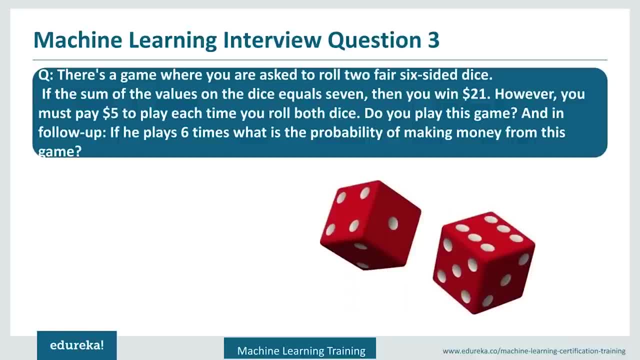 of it, we win one game of $21 and five games we lose. So in this case, for five games, we have to pay $5, and this will be $25, and we are winning one time, which is $21.. In this case, if you see, there is a 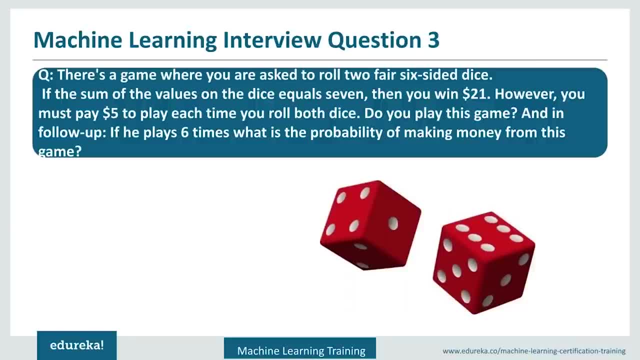 loss. So we are paying $25 and we are winning $21 in this case. So for the first question: do you play this game? this is no, As we are getting a loss as per the probability. The second question says: what is the probability of making? 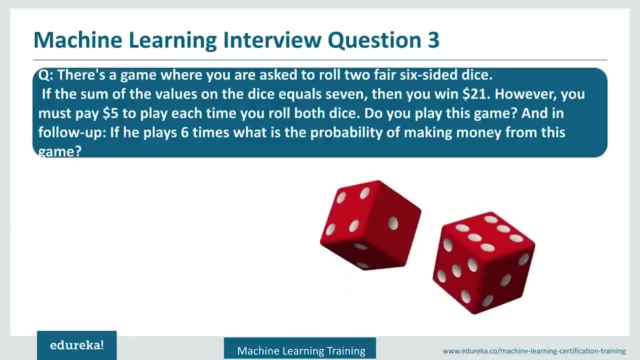 money from this game when you are playing it for six times. If you assume in this case we are making six games and out of that the winning probability, if we just have a win in one case, it be a loss. If we win two games out of six, we are going to. 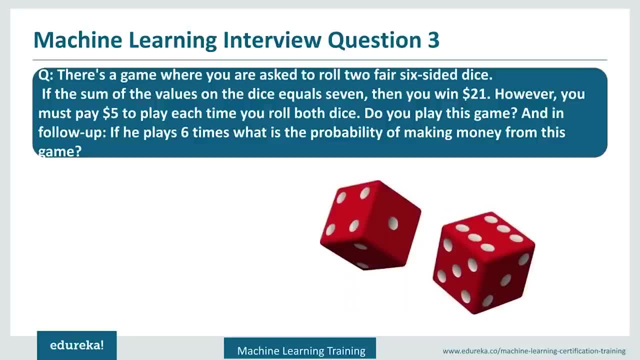 us 1 by 6 ratio. so this says we have a chance of winning 21 dollars 1 in 6 games. so assume that we are playing 6 games and out of it we win 1 game of 21 dollar and 5 games we lose. so in this, 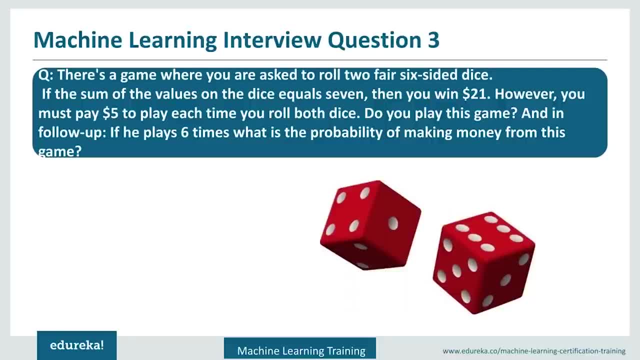 case, for 5 games, we have to pay 5 dollar, and this will be 25 dollar, and we are winning one time, which is 21 dollar in this case, if you see there is a loss. so we are paying 25 dollar and we are winning 21 dollars in this case. so for the first question: do you play this game? this is no, as we 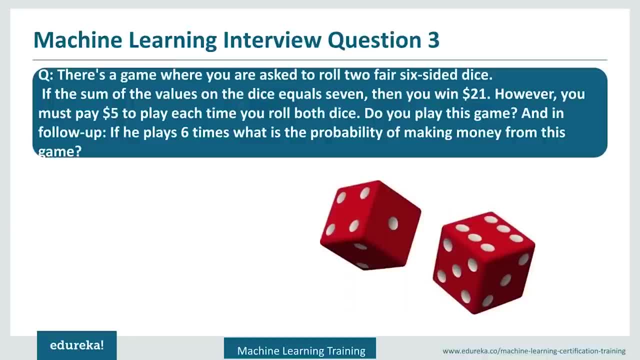 are getting a loss as per the probability. the second question says: what is the probability of making money from this game when you are playing it for 6 times? if you assume in this case we are making 6 games and out of that the winning probability, if we just have a win in one? 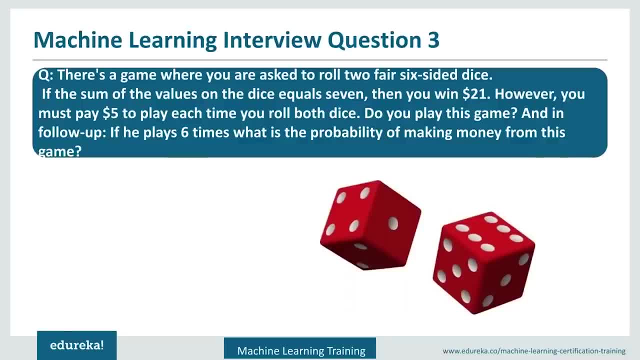 case it be a loss. if we win 2 games out of 6, we are going to win. if we win 3 games, it will be profitable again. so 2, 3, 4, 5, 6 are the cases where we will see a profit. so this case. 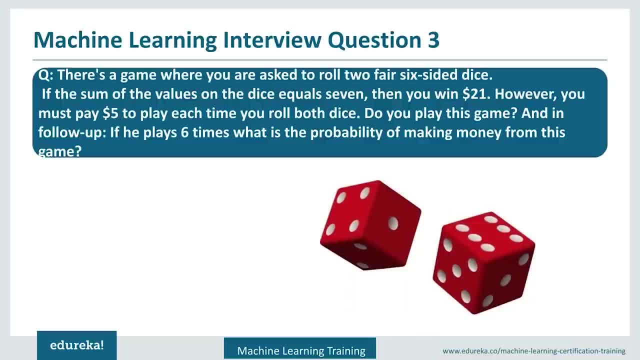 can be simulated with the binomial distribution. so binomial distribution takes three parameters. first is your probability of winning and losing, so that is, in our case, nothing but 1 by 6. the second is the number of plays, which is 6, and the third is the number of cases that we want to. 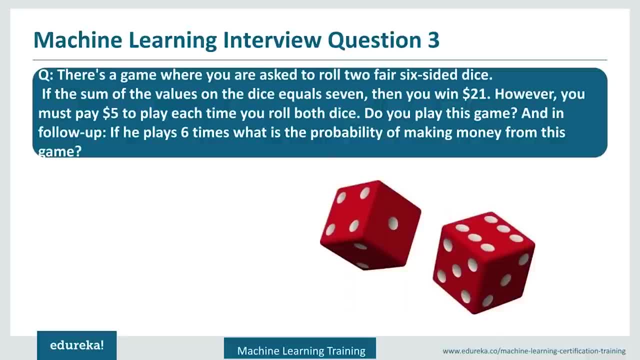 identify. so, for example, in our case we are making 1 by 6 and out of that the winning probability, if we want to have a condition where the number of wins is greater than 2. so we want to identify: the first case is a failure, where in the first case we are always losing, but in this second, if 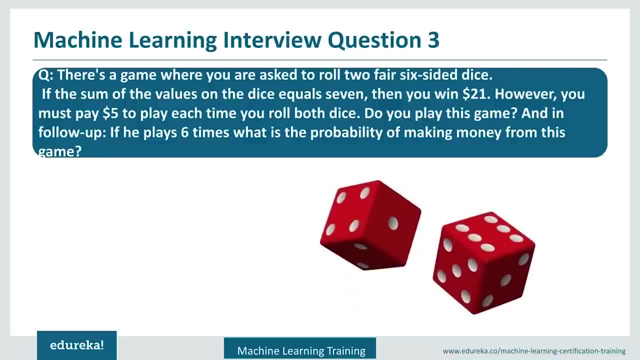 we win 2, 3, 4, 5, 6 times, we will always be winning. we will have a extra money. we have to find a probability where we will have more than two wins so that can be simulated with the probability to get the answer for this second question. so the next question. we have two options for serving. 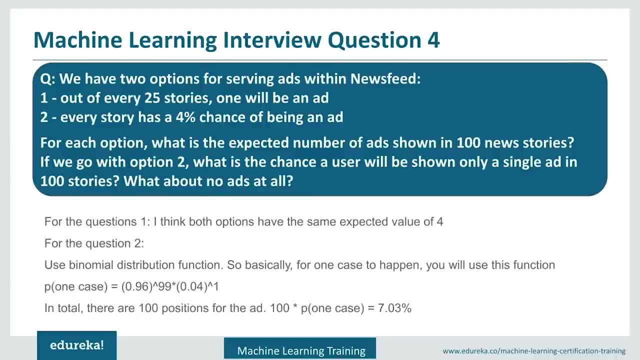 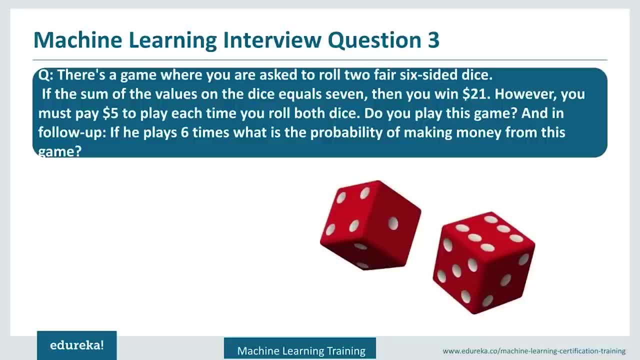 win. If we win three games, it will be profitable again. So two, three, four, five, six are the cases where we will see a profit. So this case can be simulated with the binomial distribution. So binomial distribution takes three parameters. First is 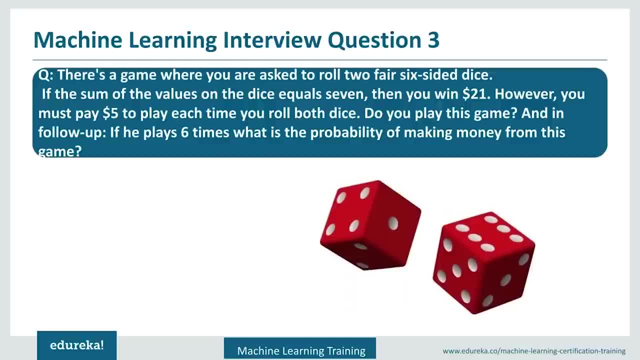 your probability of winning and losing. So that is, in our case, nothing but one by six. The second is the number of plays, which is six, and the third is the number of cases that we want to identify. So, for example, in our case, we want to have a condition. 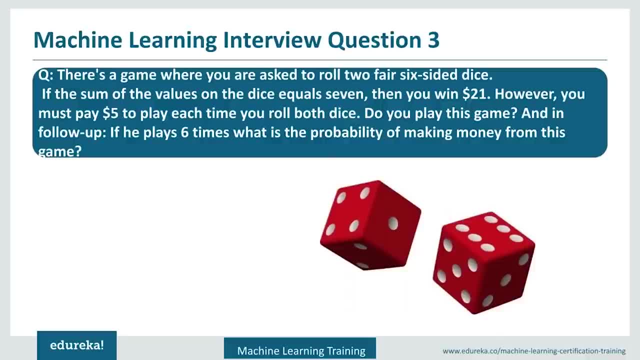 where the number of wins is greater than two. So we want to identify: the first case is a failure, where in the first case we are always losing, but in the second, if we win two, three, four, five, six times, we will always be winning. We will have a extra money We have. 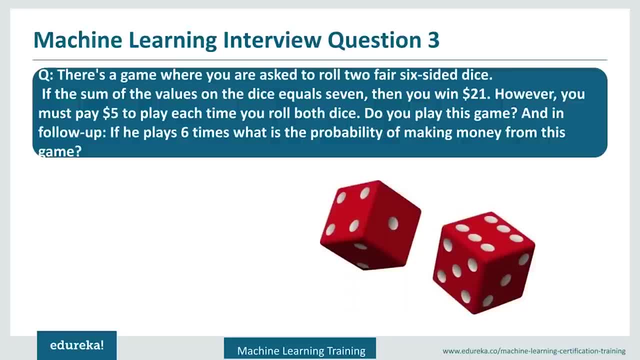 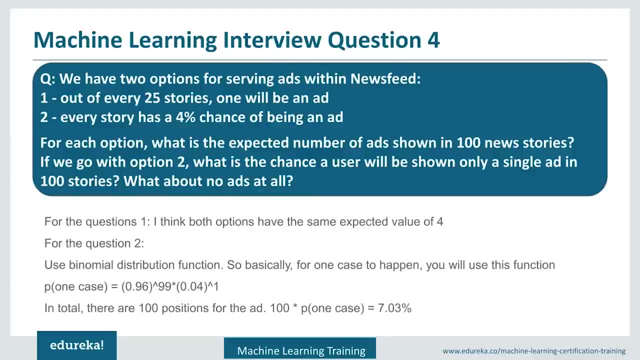 to find a probability where we will have more than two wins, So that can be simulated with the probability to get the answer for this second question. So the next question. we have two options for serving ads with newsfeed. So first is: out of every 25. 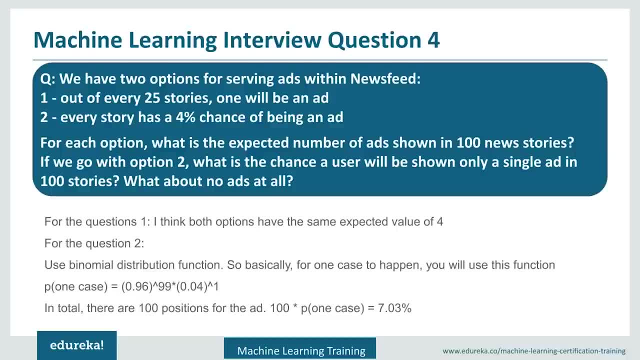 stories. one will be an ad. second is: every story has a four percent chance of being an ad. The question says for each option, what is the expected number of ads shown in hundred new stories? If we go with the option two, what is the chance a user will be? 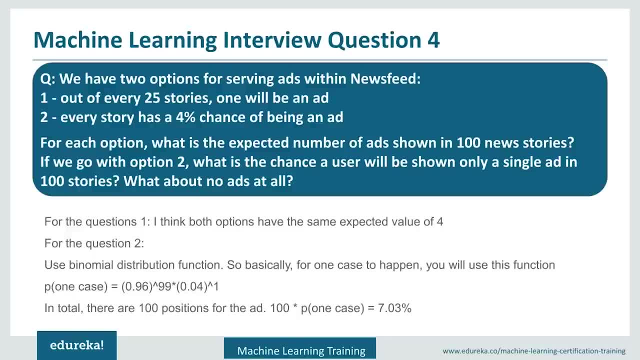 shown only a single ad in hundred stories. What about no ads at all? So in this question, if we look at the first part, which says for each option, what is the expected number of ads shown in hundred new stories? So let's check it for the first one. So for 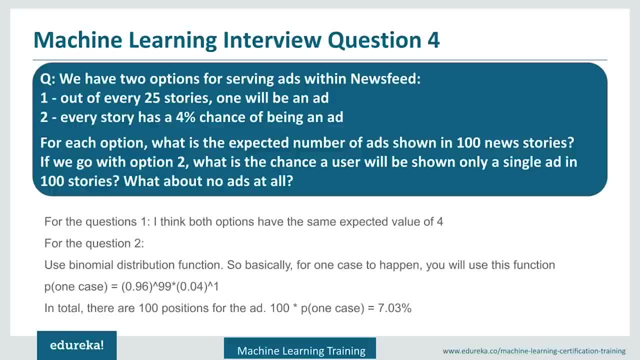 the first one: out of every 25 stories, one will be an ad, So this is like one out of 25.. In the second case, every story has four percent chance of being an ad. So this is like four out of hundred, and which is again nothing. but when we divide four. 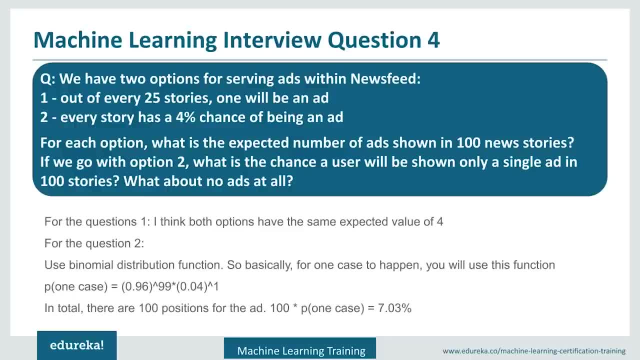 by hundred, we will have one by 25.. So for the first question the answer is: both are similar. So both the cases have expected number of ads in hundred similar, which is one by 25 or four percent. Both are equivalent to each other. For the second, 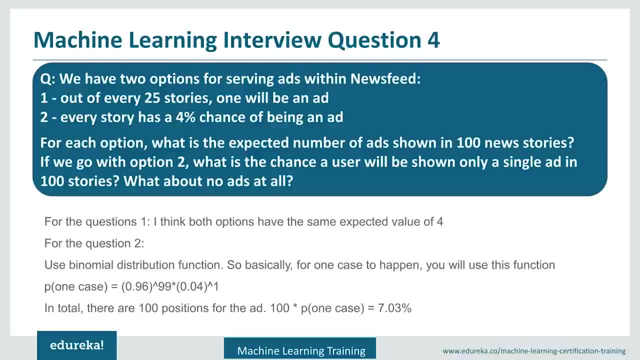 every story has a 4% chance of being an ad. the question says for each option: what is the expected number of ads shown in hundred new stories? if we go with the option 2, what is the chance a user will be shown only a single ad in hundred? 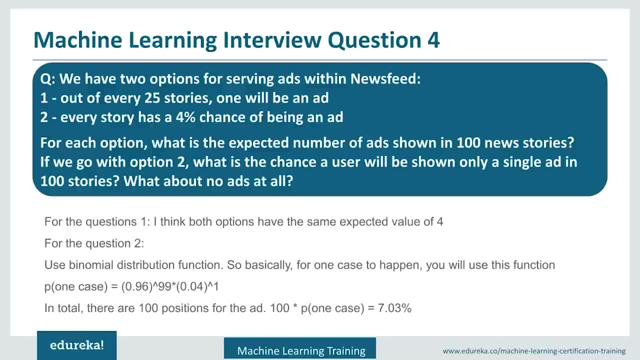 stories. what about no ads at all? so in this question, if we look at the first part, which says for each option, what is the expected number of ads shown in hundred new stories? so let's check it for the first one, so for the first one, out of every 25 stories one will be an ad. so this is like one out of 25 in the 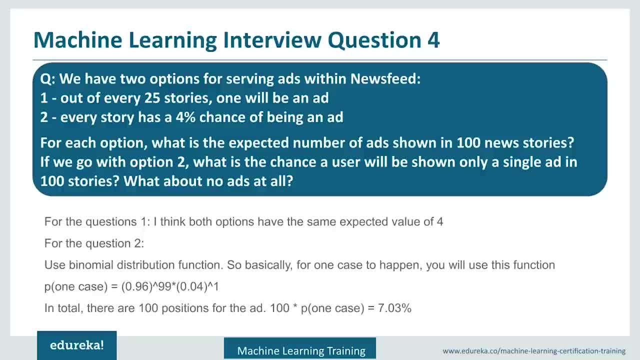 second case, every story has 4% chance of being an ad. so this is like 4 out of 100, and which is again nothing. but when we divide 4 by 100, we will have 1 by 25. so for the first question, the answer is: 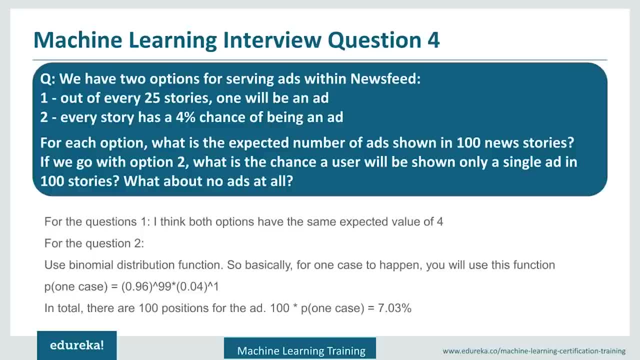 both are similar, so both the cases have expected number of ads in hundred similar, which is 1 by 25 or 4 percent. both are equivalent to each other. for the second question you have to see is the question ask: what is the chance a user will be showncom possono andare di video que uma deparare Oi. 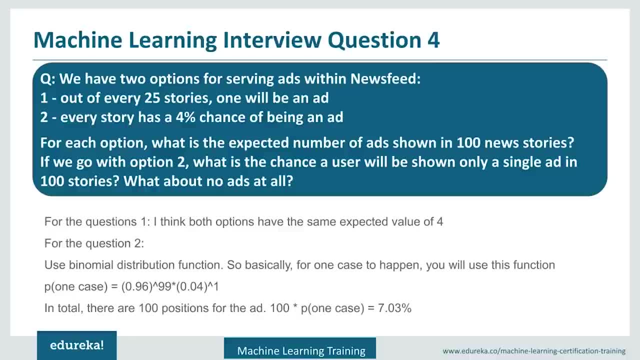 the question ask: what is the chance a user will be shown only a single ad in? shown only a single ad in 100 stories? if you see this question, it is an example of binomial distribution. so, as we just saw in the question 3, binomial distribution takes three parameters. 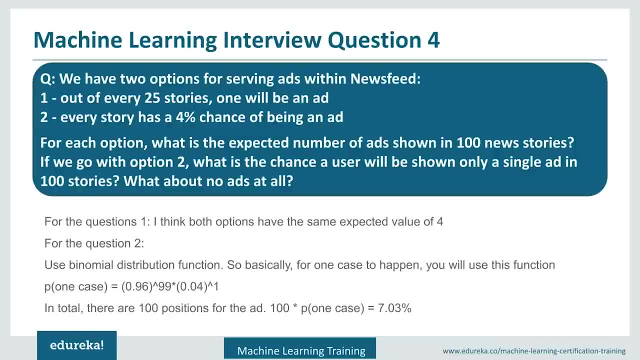 first is the probability of success and failure, which is, in our cases, four percent. second is the number of total cases, which, as the question says, 100 stories. last is the case that we want to identify, means a probability that we want to find out. so the question says: what is the? 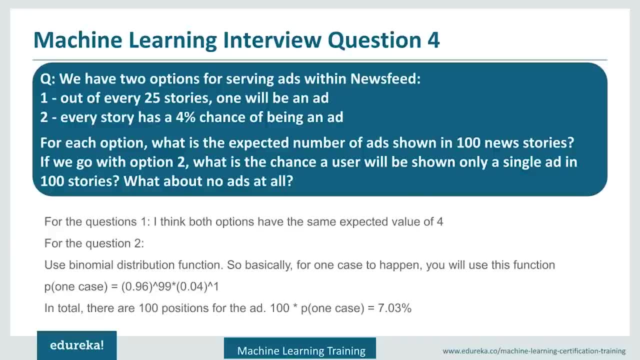 chance. a user will be shown only a single ad in 100 stories. so we want to have the three parameters as four percent hundred stories, other n and single add as our probability chance. so if you see the probability can be calculated as 0.96 is basically not getting selected, which is 1 minus 0.96. 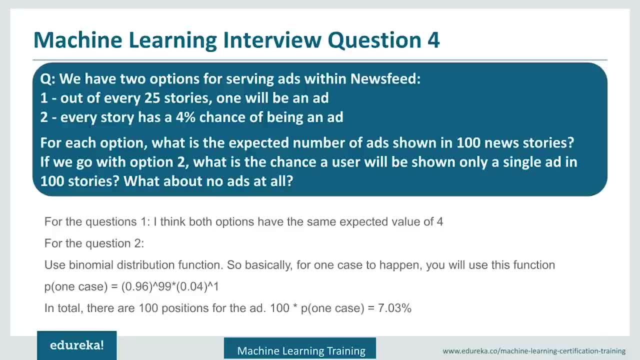 question you have to see is the question ask: what is the chance a user will be shown only a single ad in hundred stories? If you see this question, it is an example of binomial distribution. So, as we just saw in the question three, binomial distribution takes: 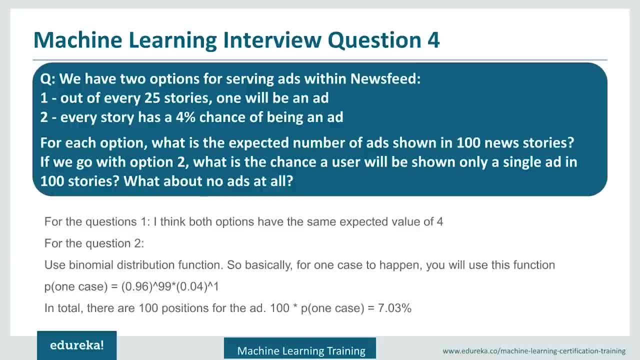 three parameters. First is the probability of success and failure, which is, in our cases, four percent. Second is the number of total cases, which, as the question says, hundred stories. Last is the case that we want to identify means, probability that we want to find out. 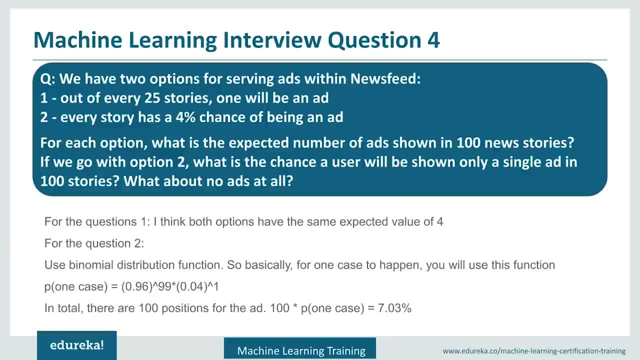 So the question says: what is the chance a user will be shown only a single ad in hundred stories. So we want to have the three parameters as four percent: hundred stories as our n and single ad as our probability chance. So if you see the probability, 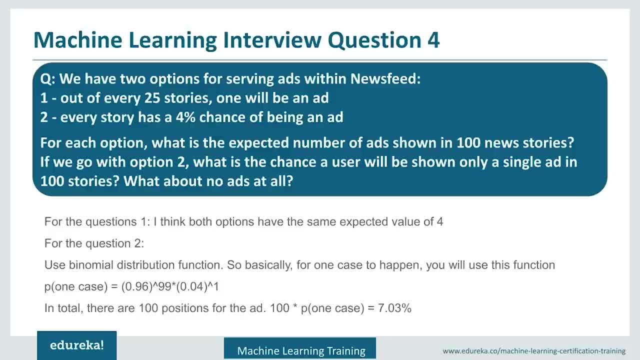 can be calculated as zero point. ninety six is basically not getting selected, which is one minus zero point. ninety six raised to nine nine, So ninety nine cases are not going to selected. multiply the chance of selecting, which is zero point zero four raised to one. So we are calculating. 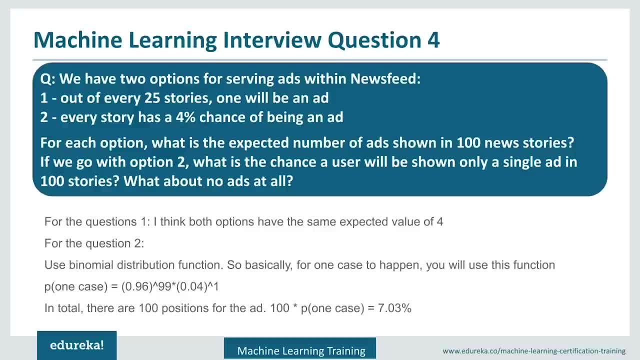 a probability of not getting selected of ninety nine samples and getting selected of one sample. So this is the binomial distribution for selecting one ad out of hundred stories. The second question just says what is the probability of no ad at all. So in that, 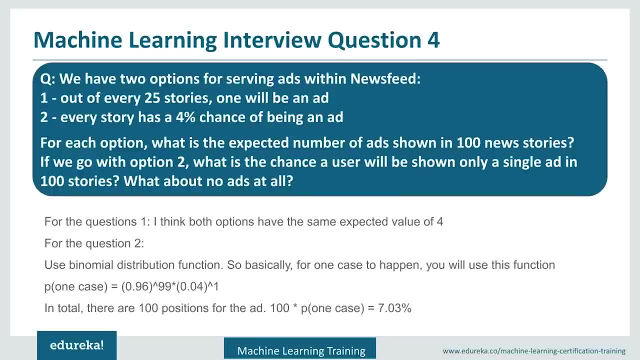 case zero and ninety nine would become hundred. So hundred multiplied by probability of one case, So it will become seven point zero, three percent. The only thing is you have to identify like which distribution is highlighted from your question. So sometimes you will see that normal distribution kind of questions. 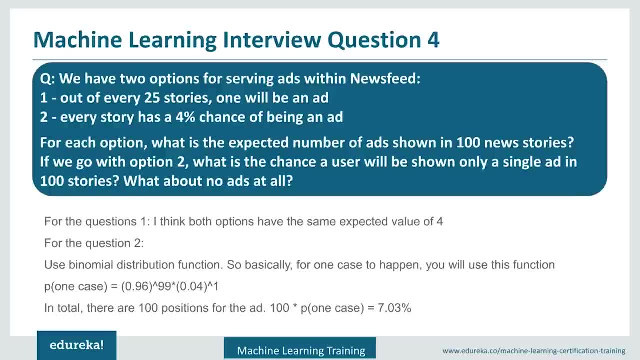 will be there where you have mean standard deviation and based on that you have to identify different things. In this case it was binomial, so based on the parameters which are there in your question, you have to identify which distribution you can use for that and try to solve it. 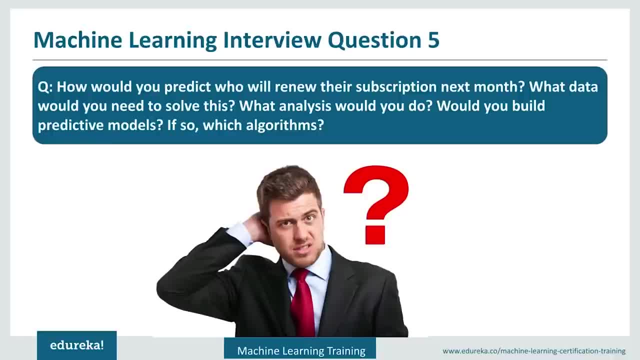 How would you predict who will renew their subscription next month? What data would you need to solve this? What analysis would you do? Would you build predictive models? If so, which algorithm would you use? This question is very generic and interviewer is really trying to understand. 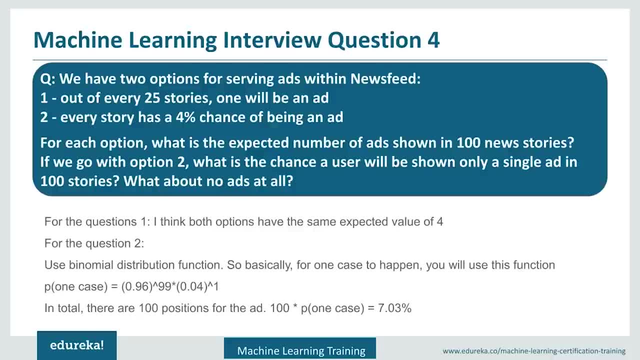 raised to 99, so 99 cases are not going to selected. multiply the chance of selecting, which is 0.04, raised to 1.. so we are calculating a probability of not getting selected of 99 samples and getting selected of one sample. so this is the binomial distribution for selecting one ad out of 100. 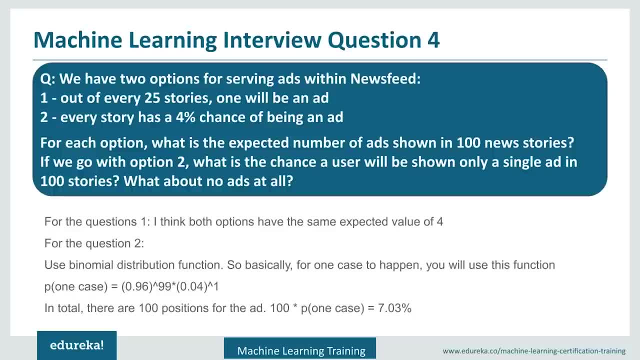 stories. the second question just says what is the probability of no ad at all. so in that case 0 and 99 would become 100.. so 100 multiply by probability of 1 case, so it will become 7.03 percent. the only thing is you have to. 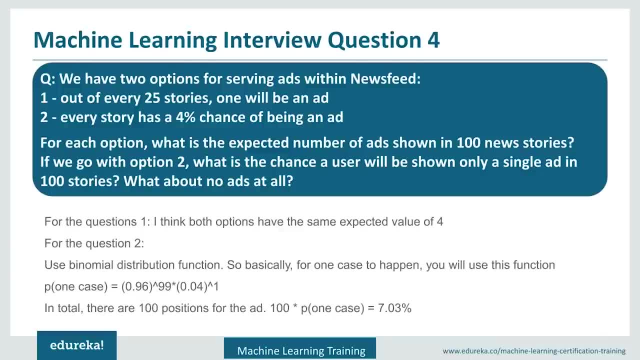 identify like which distribution is highlighted from your question. so sometimes you will see that normal distribution kind of questions will be there where you have mean standard deviation and based on that you have to identify different things. in this case it was binomial, so based on the parameters which are there in your question, you have to identify which distribution you can. 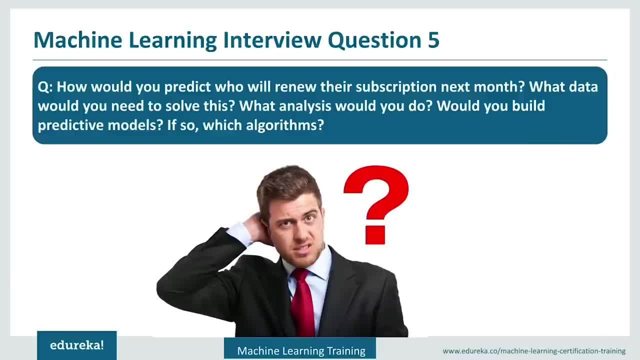 use for that and try to solve it. how would you predict who will renew their subscription next month? what data would you need to solve this? what analysis would you do? who do you build predictive models? if so, which algorithms? this question is very generic and interviewer is really trying to understand how you try to approach your problem. so when you are given a problem, 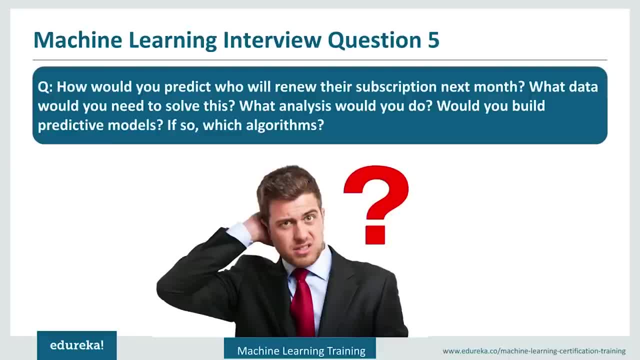 how you try to identify different components which are there within your problem. you have to solve each of those confidently, as how much of your knowledge is there within each of it? so what you have to do is: let's assume something as first thing. how would you predict who will? 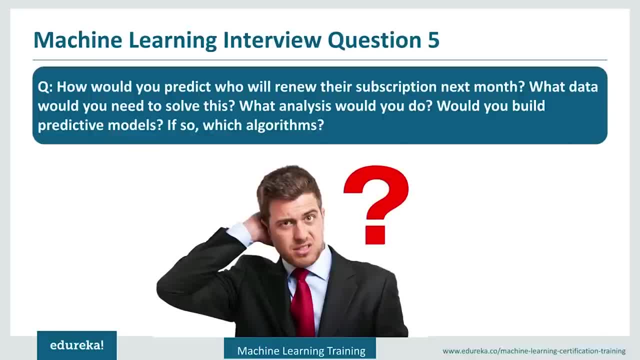 renew the subscription next month. let's assume we are trying to predict the subscription for dish tv subscription. so who is going to renew the subscription next month for the dish tv? so that is the problem statement. first we define it. what data would you need to solve this? so in the case of 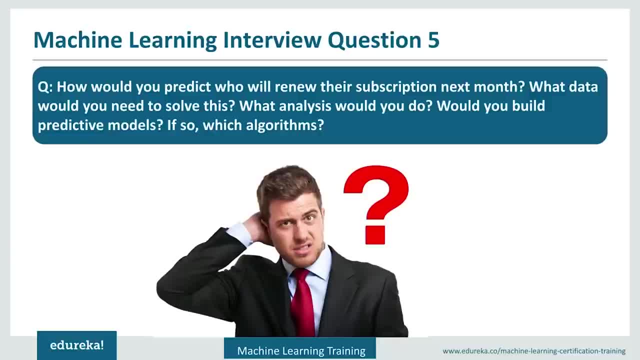 dish tv subscription. we would like to identify how many number of hours for that household the channels are active, how many number of kids are there in the home, how many number of adults are there in the home, which are the different channels they use, for how much time and from previous month. 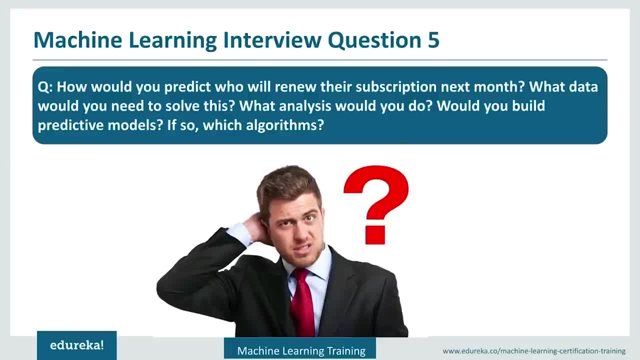 how you try to approach your problem. So, when you are given a problem, how you try to identify different components which are there within your problem, How you try to solve each of those confidently, as how much of your knowledge is there within each of it. So what you have to do is 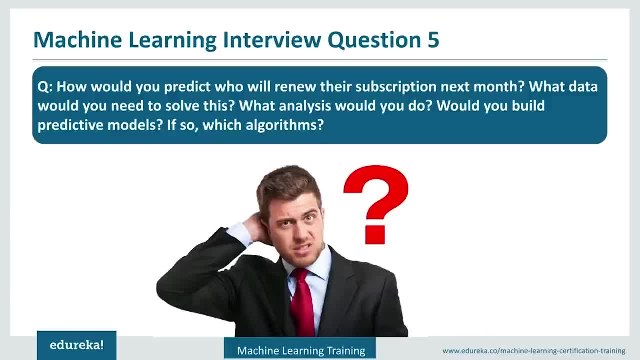 let's assume something as first thing, how would you predict who will renew their subscription next month? Let's assume we are trying to predict the subscription for dish TV subscription. So who is going to renew their subscription next month for their dish TV? So that is the 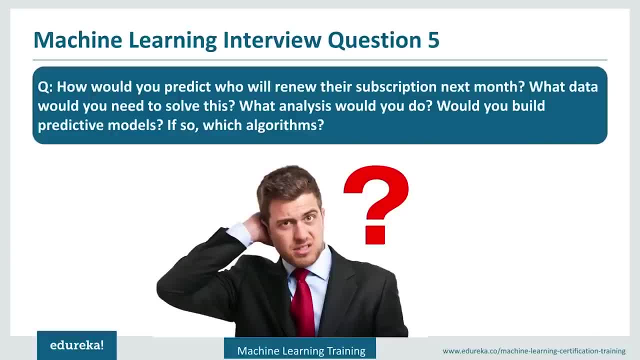 problem statement. first we define it. What data would you need to solve this? So, in the case of dish TV subscription, we would like to identify how many number of hours for that household the channels are active. How many number of kids are there in the home? 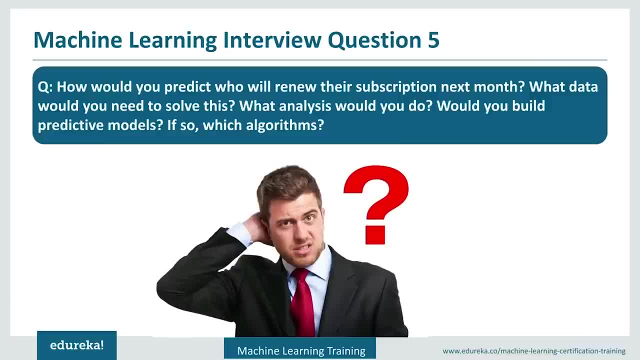 How many number of adults are there in the home, Which are the different channels they use, for how much time, and from previous month, how much increase or decrease has happened in this month. So this, all variables, would help you to understand if in the next month again, 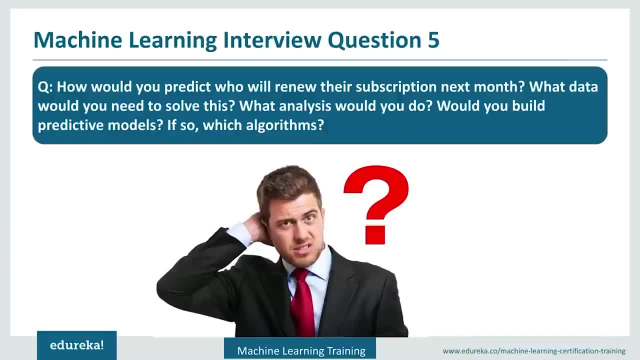 that customer is going to buy or not. So if there are kids in the home, there are chances that because of kids, whenever there are kids, they will look for the TV and kids will always help you in understanding if there will be subscription or not. And 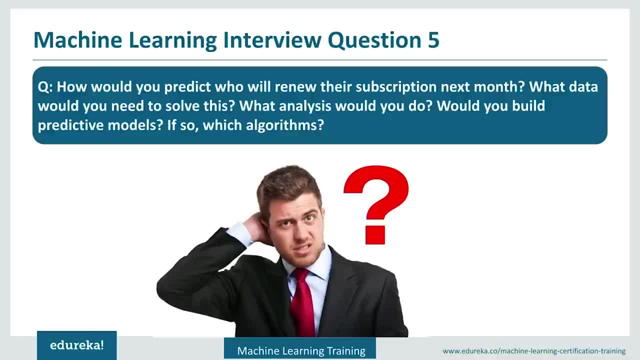 if the subscription has either increased or decreased from the previous month will also help you to understand if that user usage has increased or decreased. So that will help you to understand the trend and make your prediction better. So what analysis would you do So we? 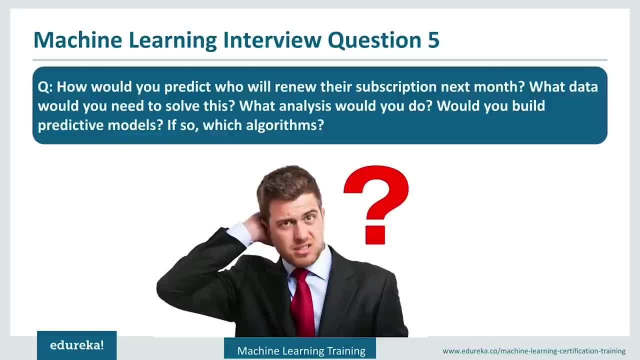 would like to do the classification analysis. in this case, We want to identify: okay, this customer is going to subscribe next month. this customer is not going to subscribe, So this is a pure classification related problem. Would you build predictive models? Yes, So before the classification related. 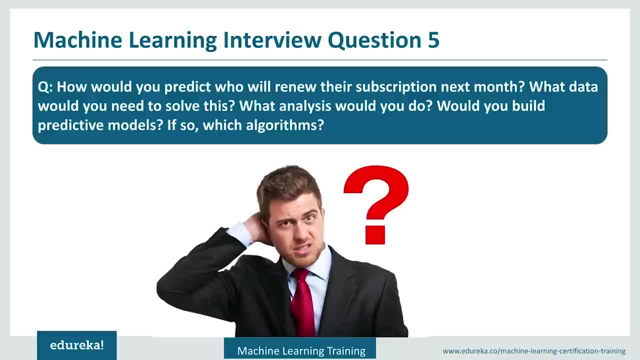 problem. we would like to build a predictive model, So we would already have a historical data. We will gather the data which is already existing and use that to train our model. So we can use any algorithm, So we can use any classification related algorithms in this case. So we 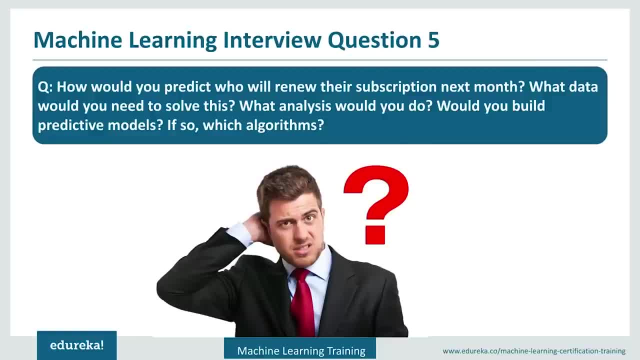 how much increase or decrease has happened in this month. so this, all variables- would help you to understand if in the next month again, that customer is going to buy or not. so if there are kids in the home, there are chances that because of kids- whenever there are kids, they will look. 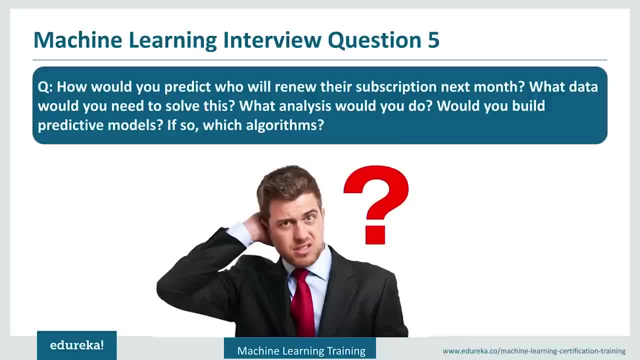 for the tv and kids will always help you in understanding if there will be subscription or not and if the subscription has either increased or decreased from the previous month will also help you to understand if that user usage has increased or decreased. so that will help you to understand. 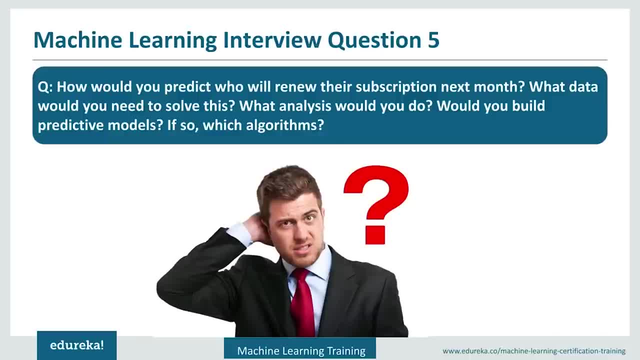 the trend and make your prediction better. so what analysis would you do? so we would like to do the classification analysis. in this case, we want to identify: okay, this customer is going to subscribe next month. this customer is not going to subscribe, so this is a pure classification related problem. 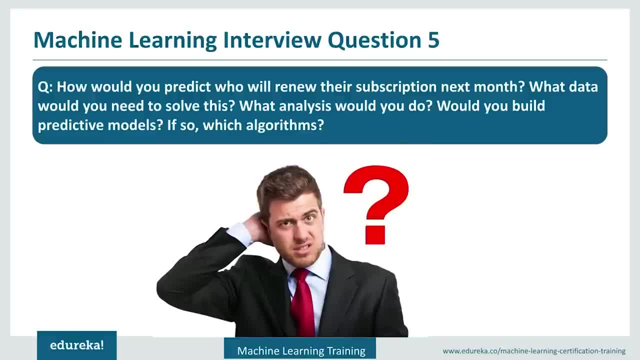 would you build predictive models? yes, so before the classification related problem, we would like to build a predictive model so we would already have a historical data. we will gather the data which is already there, already existing, and use that to train our model. so we can use any algorithm, so we can use any. 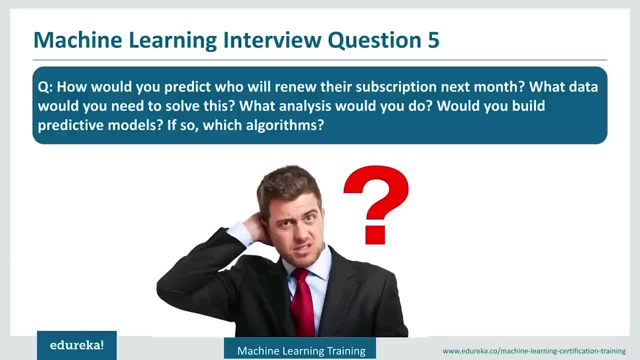 classification related algorithms in this case. so we can use random forest, we can use logistic regression, we can use neural networks- whichever, we can try different models and see which one performs better and based on that, we can continue with the model which performs better and tune it further. so you have to start with this step by step and show that. okay, this is the next step. 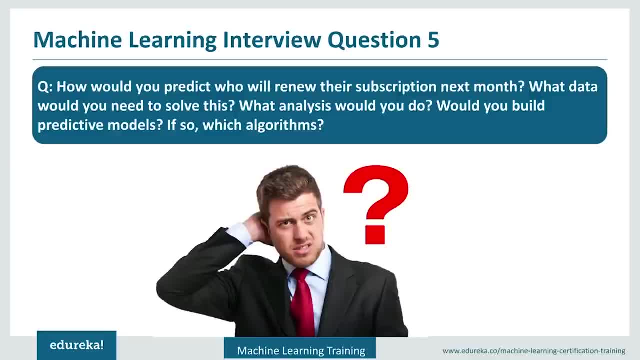 this is the next step till the end of your model. so even in this case, if so, which algorithm would not end the problem algorithm you have selected? after that, you have to validate your algorithm. it will even go that in production and within production you will also validate again and see in real life how it's working. make again changes to. 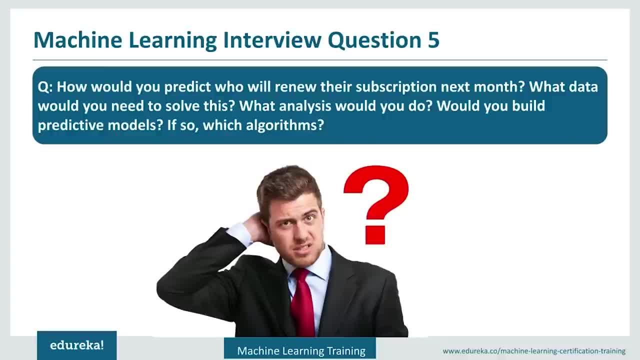 the model. so those things may change again, as the interviewer may keep on asking you the further things and you have to be ready for those things. interview may start with few questions, but as you keep on solving the problem, interview keep on digging further, as what would you do next? so you 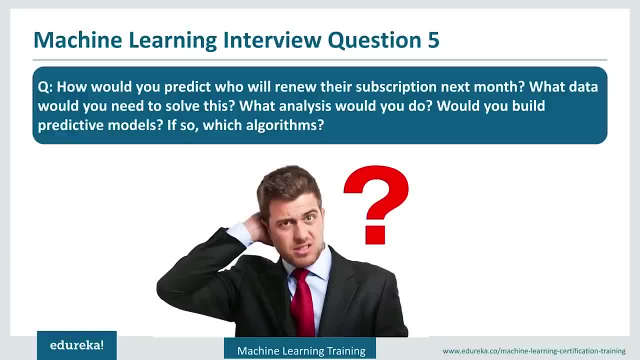 can use random forest, we can use logistic regression, we can use neural networks. whichever, we can try different models and see which one performs better and based on that, we can continue with the model which performs better and tune it further. So you have to start. 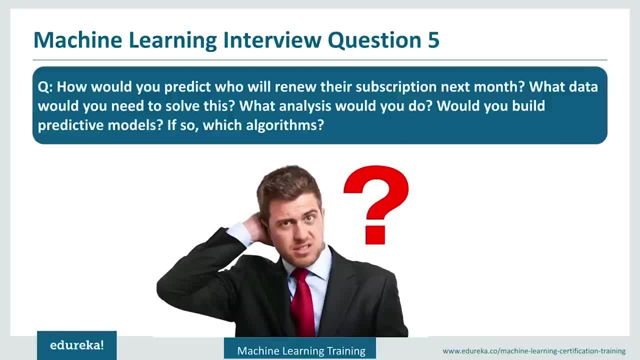 with this, step by step, and show that, okay, this is the next step, this is the next step till the end of your model. So, even in this case, if so, which algorithm would not end the problem? Algorithm you have selected. after that, you have to validate your algorithm. 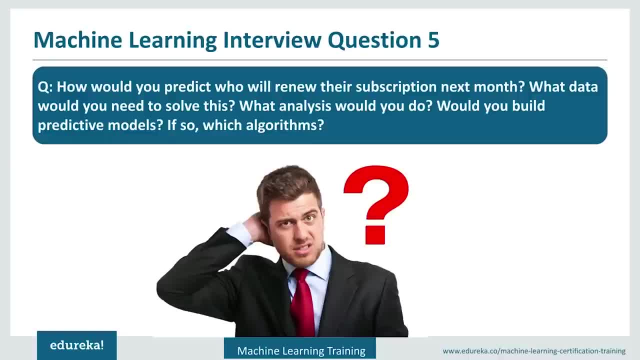 It will even go that in production and within production you will also validate again and see in real life how it's working, make again changes to the model. So those things may change again as the interviewer may keep on asking you the further things and you have to be ready for those things. 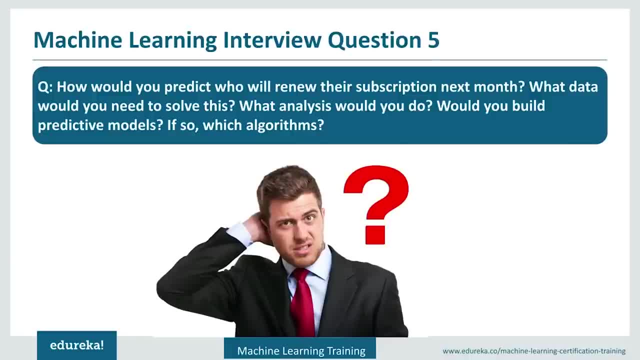 Interview may start with few questions, but as you keep on solving the problem, interviewer, keep on digging further, as what would you do next? So you have to be ready for all those things. So be prepared for those things. How do you map nicknames? Pete Andy, Nick, Rob? 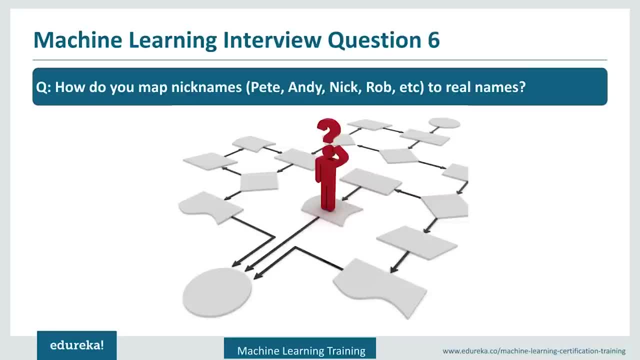 etc. to real names. So this is like understanding how you try to solve a problem where there is not much of data is there. So this example is just: you have just a nicknames and you want to identify the real names to them. So this can. 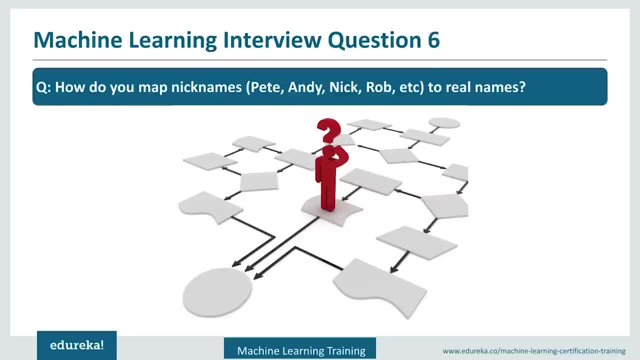 have different answers. It is not related to a single answer and there is no generic, fixed answer, but interviewer would be interested to know as how you are trying to approach the problem and solve it. So few things could be like, as you don't have any data. 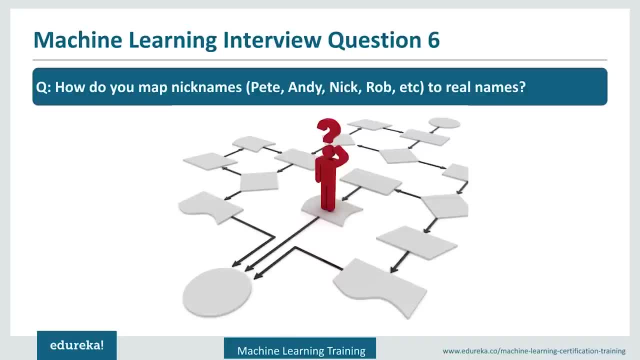 first you try to gather as to which component these things are related. So, for example, if you are trying to understand this nicknames from a Twitter tweets, try to see who is trying to refer to who and, based on this nicknames, see the relation as which person is trying to. 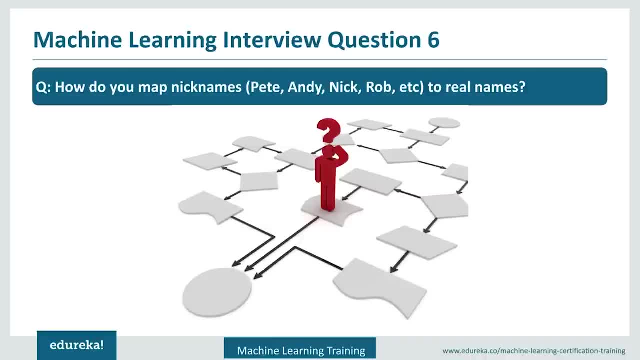 talk with which person and you can try to identify, based on the NLP algorithms, as what is the real names for those people. So, similarly, you can try to identify in the Facebook or if you have some customer feedbacks and within those customer feedbacks you want to understand this, you can. 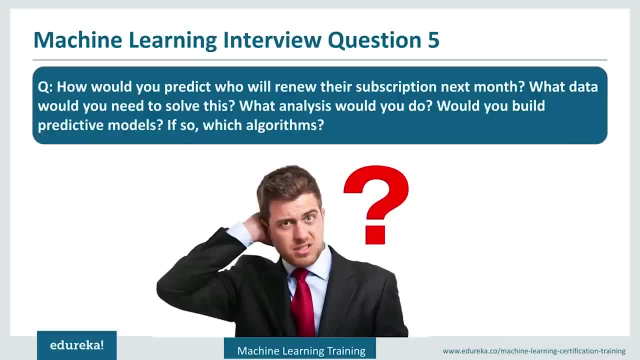 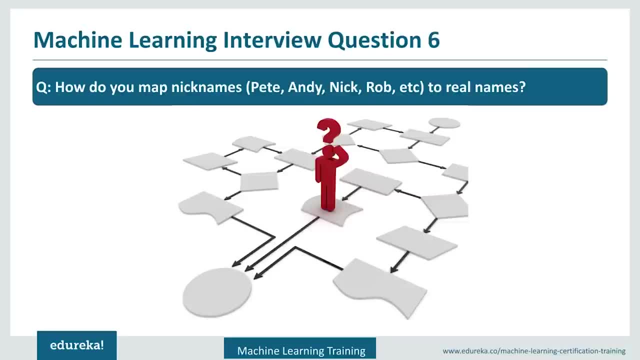 have to be ready for all those things. so be prepared for those things. how do you map nicknames- pete andy, nick, rob, etc. to real names? so this is like understanding how you try to solve a problem where there is not much of data is there. so this example is just: you have just a nicknames. 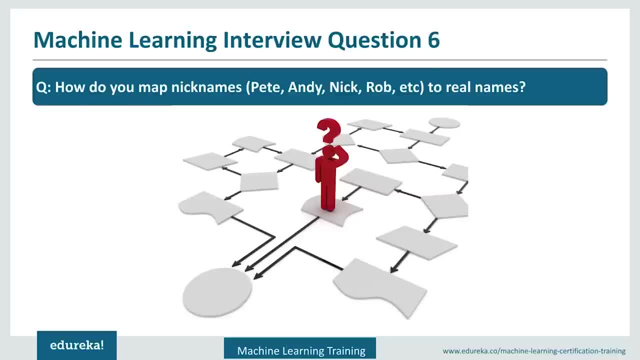 and you want to identify the real names to them. so this can have different answers. it is not related to a single answer and there is no generic, fixed answer, but interview would be interested to know as how you are trying to approach the problem and solve it. so few things could be like. as you don't have any data, first you try to gather as to which. 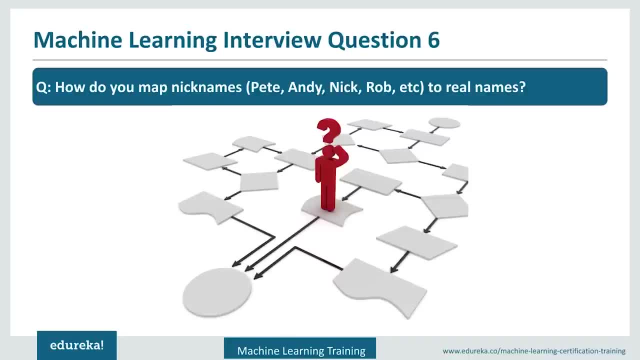 components. these things are related. so, for example, if you are trying to understand these nicknames from a twitter tweets, try to see who is trying to refer to who and, based on these nicknames, see the relation as which person is trying to talk with which person, and you can try to identify based on the nlp. 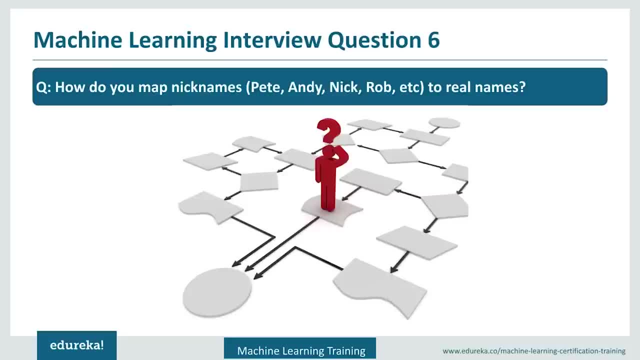 algorithms, as what is the real names for those people. so, similarly, you can try to identify in the facebook or if you have some customer feedbacks and within those customer feedbacks you want to understand this, you can do it that way, but this would be more like you have to understand. 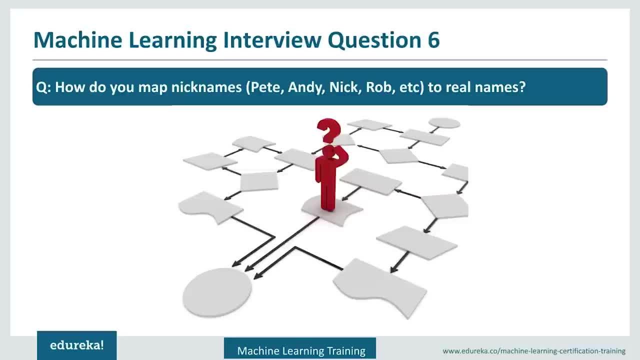 in the context, so in which context people are talking to whom, and based on that you can try to identify the real names. so this is just one example, but it is not related to just single one. you can create your own, as, as i said, there is no single. 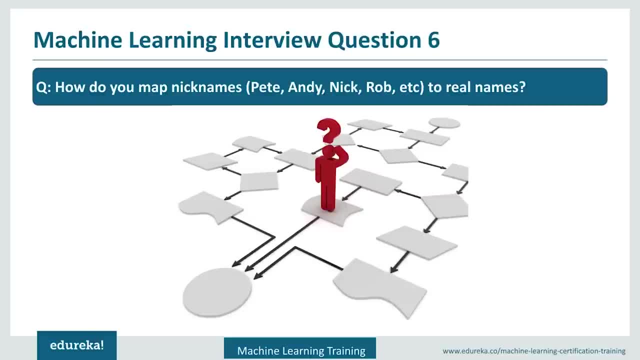 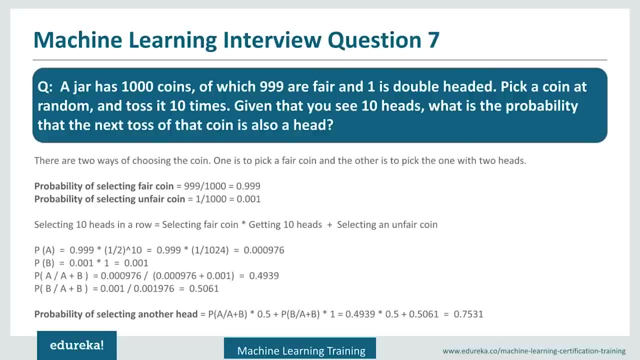 answer to this problem, but it mostly depends on how you are trying to approach that problem and solve it. a jar has thousand coins, of which 999 are fair, and one is double headed. pick a coin at random and toss it 10 times. given that you see 10 heads, what is the probability that the next toss of 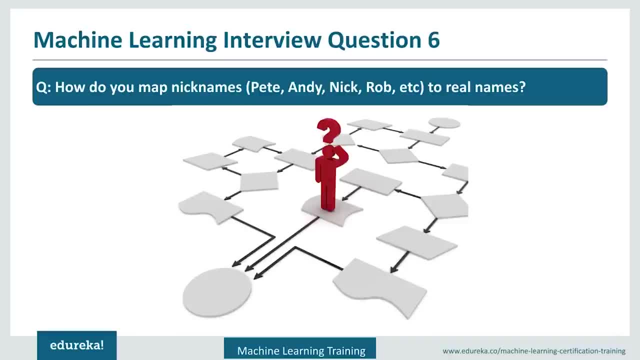 do it that way, But this would be more like you have to understand in the context, So in which context people are talking to whom, and based on that you can try to identify the real names. So this is just one example, but it is not. 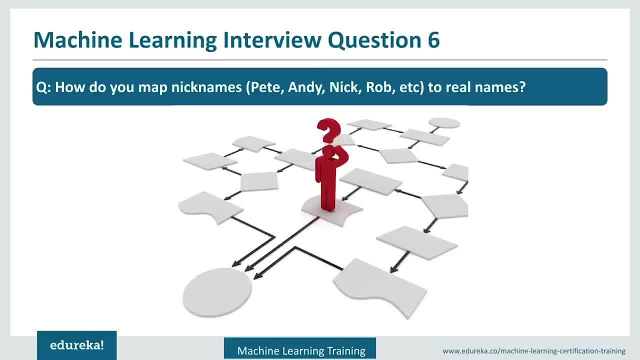 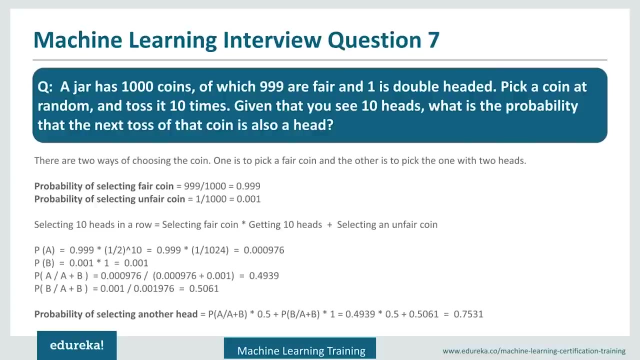 related to just single one. You can create your own. as I said, there is no single answer to this problem, but it mostly depends on how you are trying to approach that problem and solve it. A jar has thousand coins, of which 999 are fair and one is. 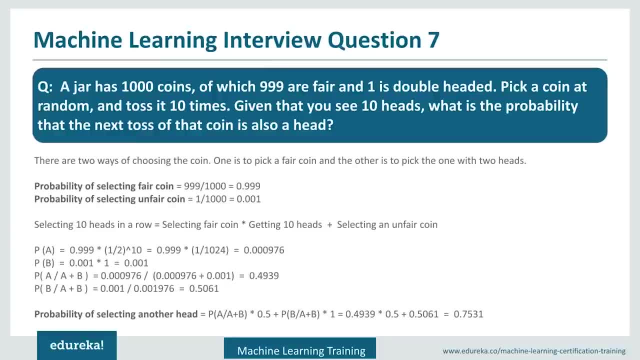 double headed. Pick a coin at random and toss it 10 times. Given that you see 10 heads, what is the probability that the next toss of that coin is also a head? So let's first try to split the problem statement that we have. So the different. 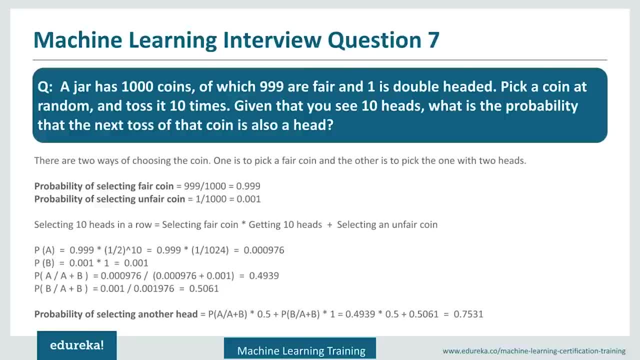 components are. we have thousand coins, of which 999 are fair. so for the fair case we can say that, okay, there is 0.5% probability that it could be head or it could be tail, And one is double headed. So it is not having probability and it is. 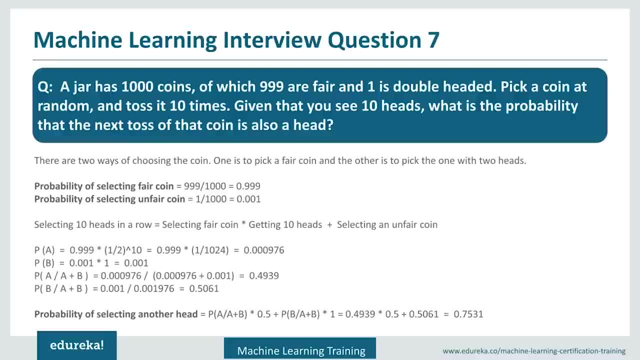 just 100% probability that it's a head. We pick a coin at random out of this thousand and toss it 10 times. So each time we select a coin, we toss it. We select a coin, we toss it. So we try to do. 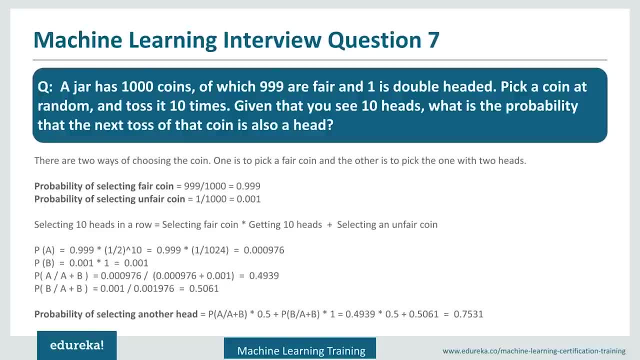 it 10 times. Given that you see 10 heads, what is the probability that the next toss of that coin is also a head? So let's see what we can do in this case. So, basically, we have two types of coin which can be chosen. 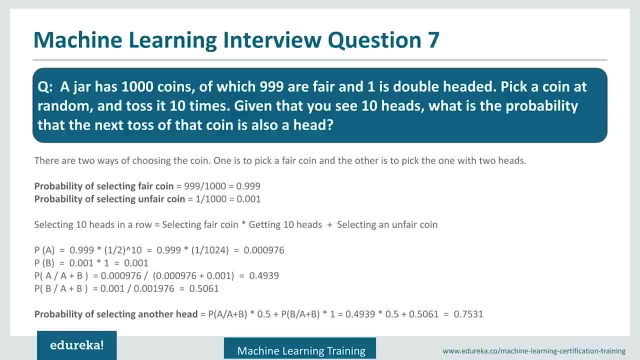 in a two different ways, basically, and there are probabilities associated with each and they are different. So, for the first type of coin, which is fair, we have 999 out of 1000, so which is 0.999, and this chances of selecting the second coin, which is unfair. 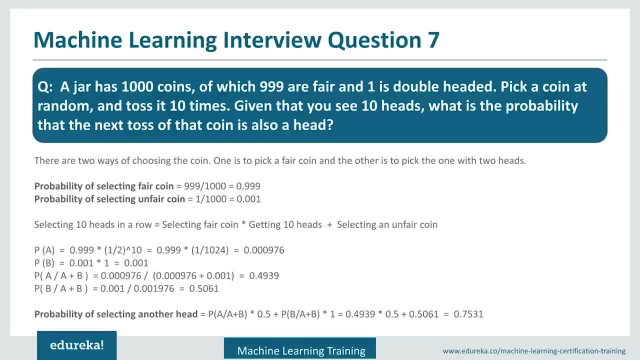 in nature is 1 out of 1000.. So these are the probabilities that we have got first. Now, as the question says, we have already chosen 10 heads, We have already done some experiment and we have got 10 heads. So what is the probability of selecting those? 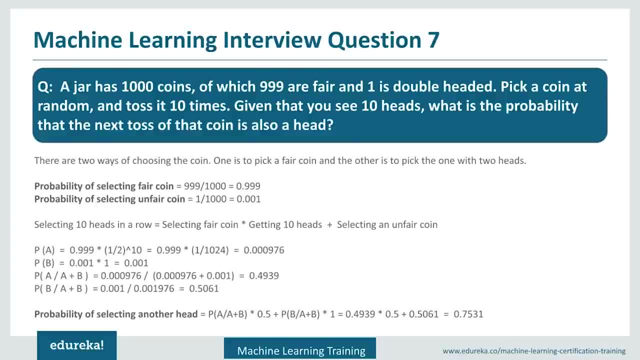 chain. two is also a head. so two heads different components are. we have thousand coins, of which 999 are fair. so for the fair case we can say that, okay, there is 0.5 percent probability that it could be head or it could be tail, and one is double-headed. so it is not having probability and 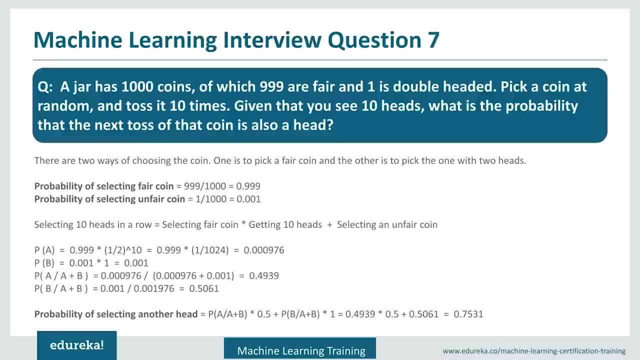 it is just 100 probability that it's the head. we pick a coin at random andplayer a 55 percent probability that it is a head. but who said that it was head? i just have to drop that one. it's not got left to тр. i just have to drop that one. it's not got left to press train so that i canrat pilgrim head river in scope. 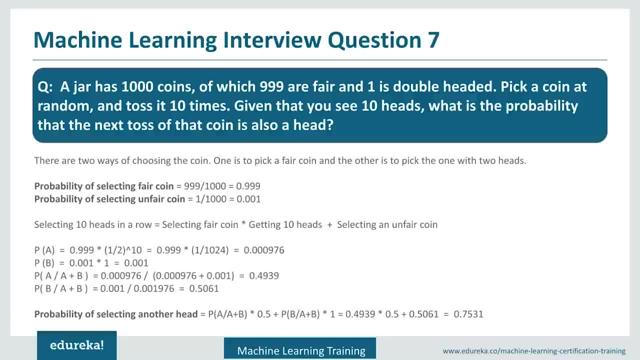 it random out of this thousand and toss it 10 times. so each time we select a coin, we toss it. we select a coin, we toss it, so we try to do it 10 times. given that you see 10 heads, what is the probability that the next toss of that coin is also a head? so let's see what we can do in this. 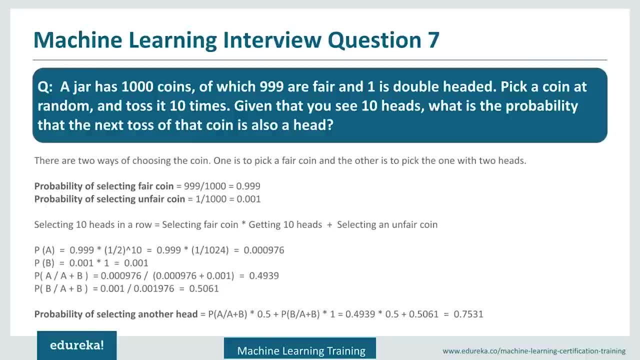 case. so, basically, we have two types of coin which can be chosen in a two different ways, basically, and there are probabilities associated with each and they are different. so, for the first type of coin, which is fair, we have 999 out of 1000, so which is 0.999, and this chances of selecting. 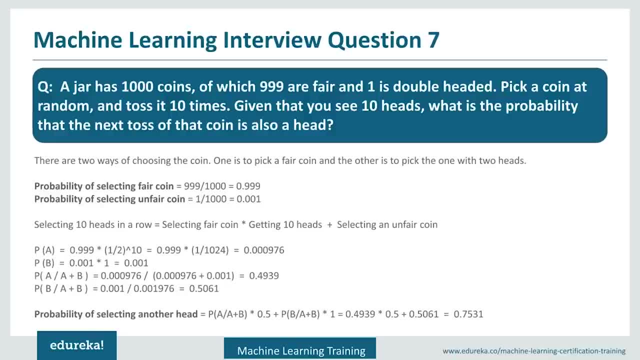 the second coin, which is unfair in nature, is one out of thousand. so these are the probabilities that we have got first. now, as the question says, we have already chosen 10 heads. we have already done some experiment and we have got 10 heads, so what is the probability of selecting those? so selecting 10 heads in a row is equal to the. 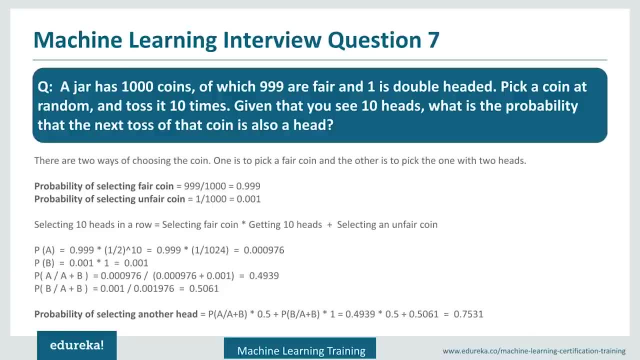 chances of selecting fair coin multiply by getting 10 heads plus selecting an unfair coin. so if we see that first thing is selecting 10 coins from the 999 fair coins is we have the probability 0.999. multiply by the fairness is basically probability 0.5 raised to 10, which will give us 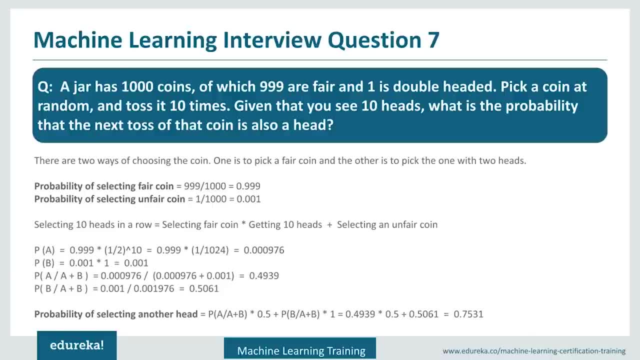 So selecting 10 heads in a row is equal to the chances of selecting fair coin. multiply by getting 10 heads plus selecting an unfair coin. So if we see that first thing is selecting 10 coins from the 999 fair coins is we have the 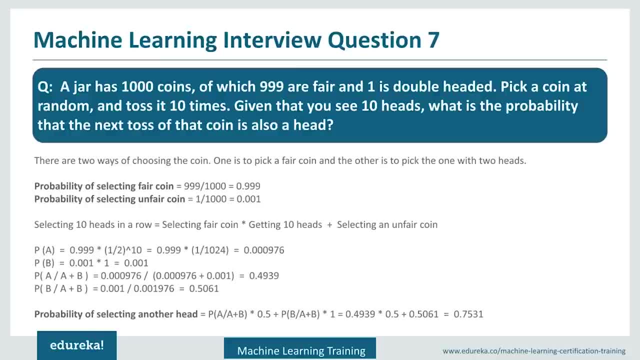 probability 0.999 multiply by the fairness is basically the probability 0.5 raise to 10, which will give us 0.999 multiply by 1 by 1024.. So when we multiply this we will get a chance of selecting coin A, which is nothing. 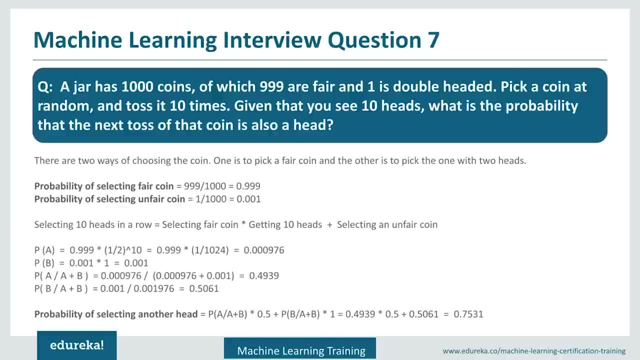 but selecting the 10 coins from the fair coins. The second part is the probability of selecting the second coin, unfair coin. multiply by 1, which is basically everything is head there. as we don't have anything, everything is head, so it is 1.. So probability. 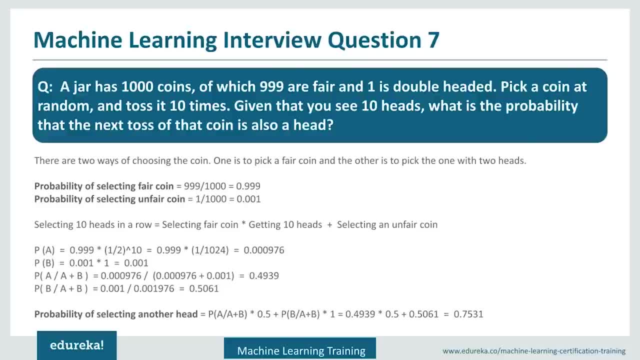 of here is 0.001.. Probability of A says selecting the 10 coins from the fair coins. Probability of B says selecting the 10 coins from the double headed ones. Now the second question says: given probability of fair coins, what is the chance of selecting the coin? 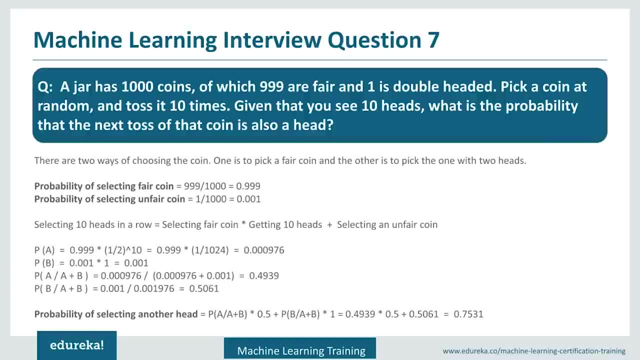 from that, It is like a conditional probability and in this conditional probability what we are doing is we are dividing the probability of A given probability of A and B. So, given both of them, what is the probability of selecting the coins from the fair coins? 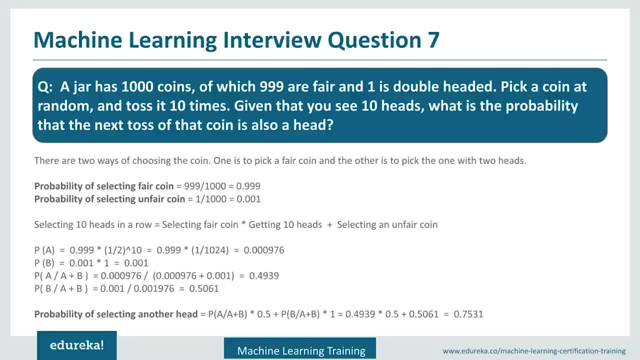 This is the probability and the second part basically says: given double headed sided coins, what is the probability of selecting from that? So these are the two individual cases. once we have got that, we have to create a combined probability which will include the chances of selecting the coin from the fair coins. 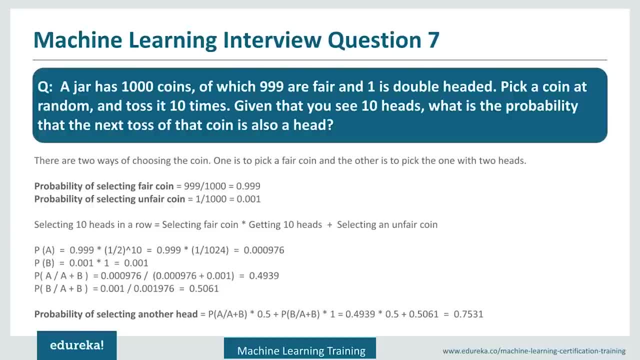 multiply by 0.5, plus the chances of selecting the coin, given it is the double headed, multiply by 1, and this would create a combined probability and give you the output as 0.7531.. So for this case we have to go step by. 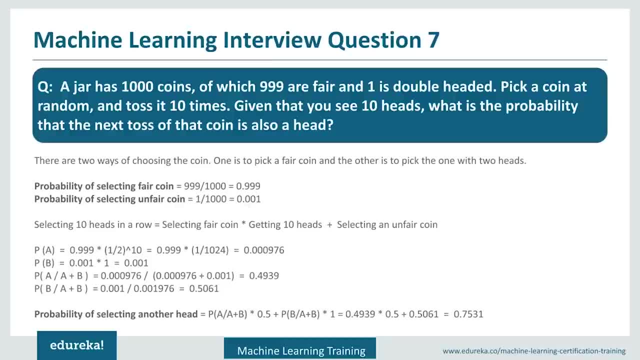 0.999 multiplied by 1, by 1024. so when we multiply this, we will get a chance of selecting coin a, which is nothing but selecting the 10 coins from the fair coins. the second part is the probability of selecting the second coin, unfair coin. multiply by 1, which is basically everything is head there. 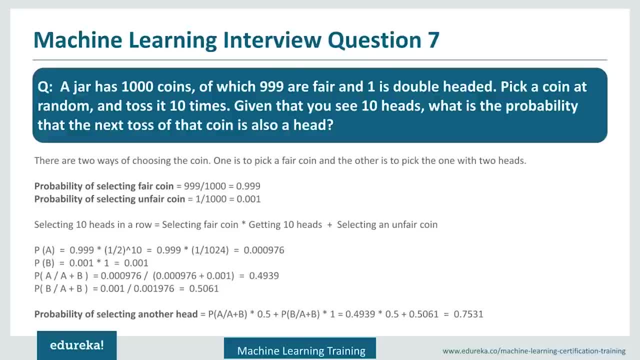 as we don't have anything, everything is head, so it is 1. so probability of here is 0.001. probability of the 10 heads and, from the fair coins, probability of bsst selecting the 10 coins from the double headed ones. now the second question says: given probability of fair coins, what is the chance of? 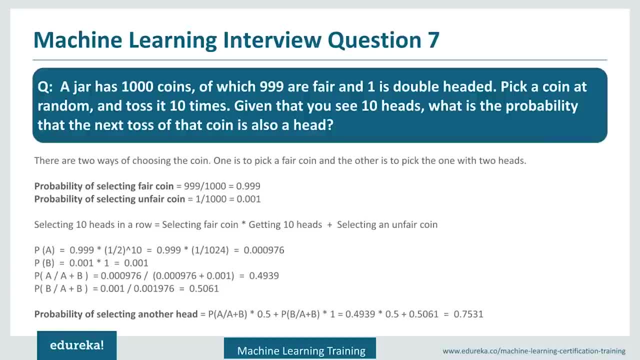 selecting a coin from that. it is like a conditional probability and in this conditional probability, what we are doing is we are dividing the probability of a given probability of a and b. so, given both of them, what is the probability of selecting the coins só, the fair coins? this is the probability and the بين false. 어떻게 вычисли 150i这种会処�? Needed to fill the 없습니다 5i ens of select, of select coins from the fair coinsill follow throughになります probability and this conditional probability, and we are dividing the probability of a given, This probability of achoadoa, according to lemme. 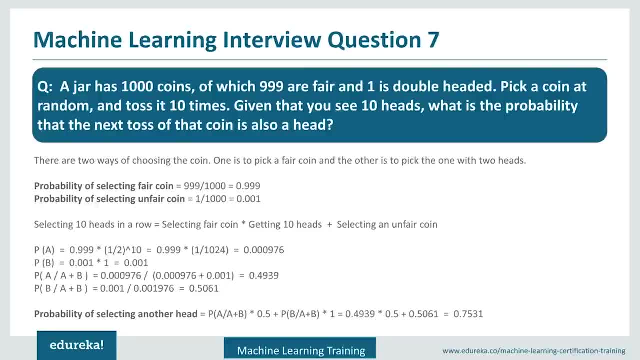 probability of shareholders problems: franc welpower when probability of coins less than 10 coins approximately. second part basically says: given double headed sided coins, what is the probability of selecting from that? so these are the two individual cases. once we have got that, we have to create a combined. 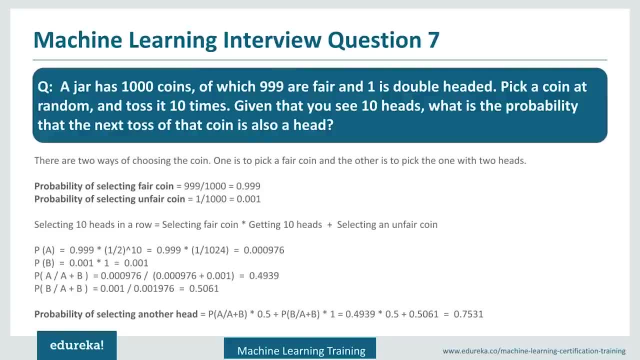 probability, which will include the chances of selecting the coin from the fair coins multiplied by 0.5, plus the chances of selecting the coin, given it is the double headed multiplied by 1, and this would create a combined probability and give you the output as 0.7531. so for this case, 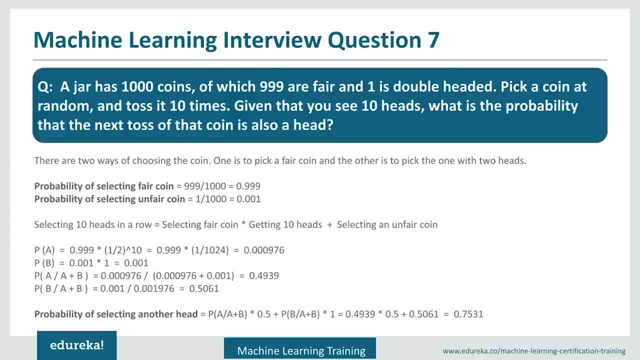 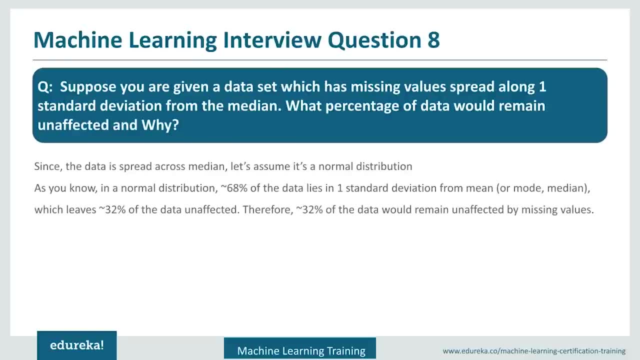 we have to go step by step, divide the problem into smaller parts and get to the answer of it. suppose you are given a data set which has missing values spread along one standard deviation from the median. what percentage of data would remain unaffected, and why? in this case, there is not much. 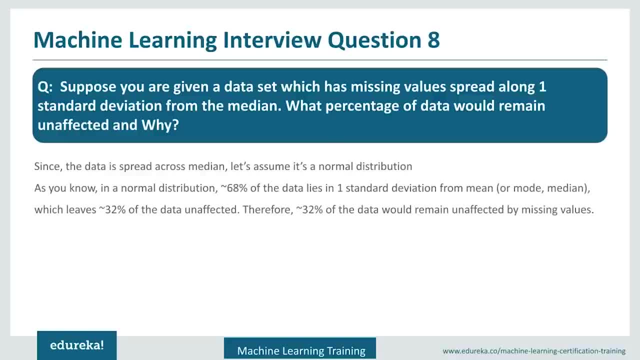 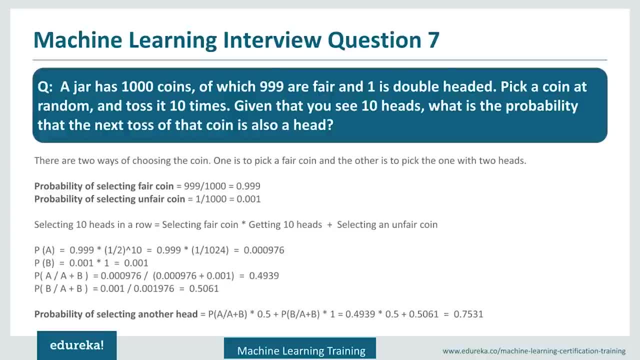 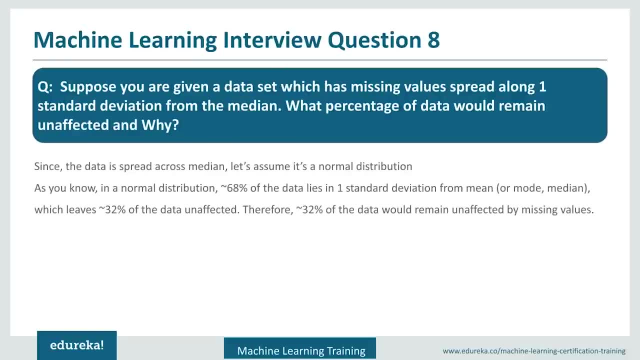 step, divide the problem into smaller parts and get to the answer of it. Suppose you are given a data set which has missing values spread along one standard deviation from the median. what percentage of data would remain unaffected, and why? In this case, there is not much. 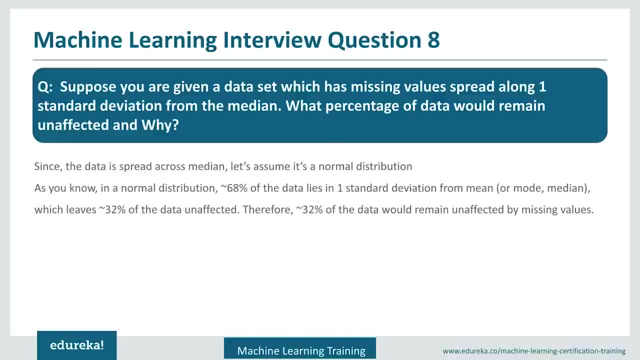 details about how is the distribution of data. It is just said that there is a one standard deviation from the mean, which is missing data, So we have to make some assumptions. so as most of the data follows a normal distribution, you would assume that this data is also following a normal. 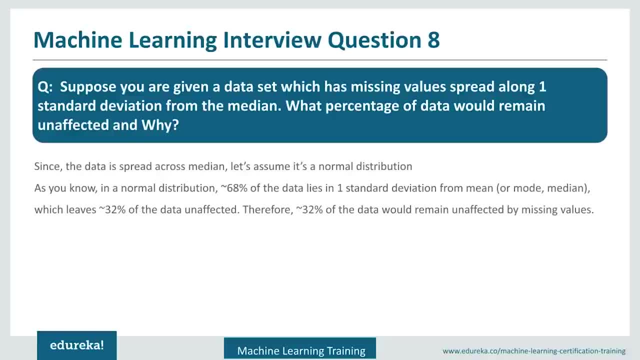 distribution and you would say that, okay, a normal distribution has, within one standard deviation, a 68% of the values. So, as per the normal distribution, within one standard deviation, around the mean median and more. as for the normal distribution, all are equal, all mean median mode are at the same location. 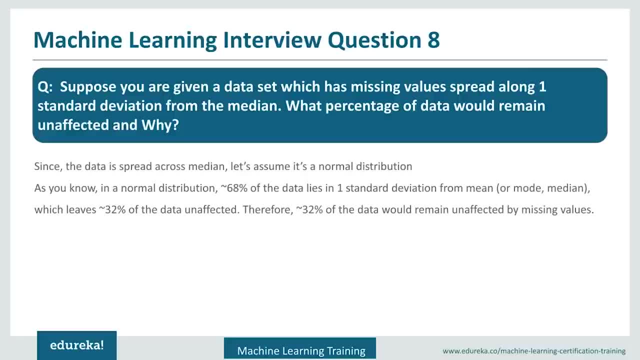 and from the mean around one standard deviation, we would have 68% of the values and, as the question says, missing values are spread along one standard deviation. so 68% of the values are basically missing and question asks what percentage of data would remain unaffected and why. 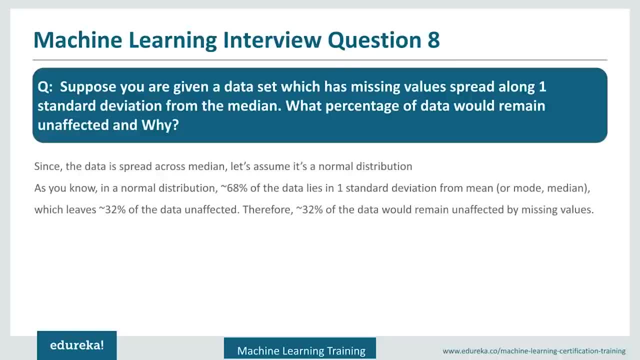 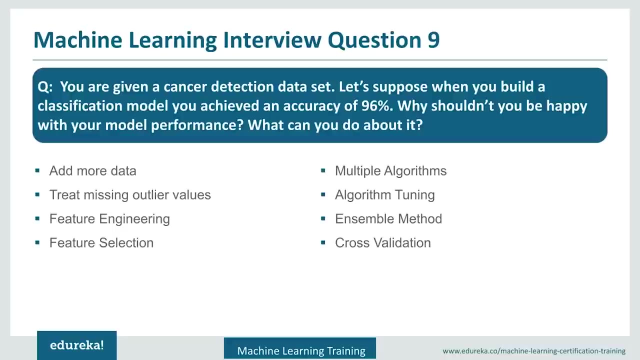 So everything left after the 68% would remain unaffected. So you would say 100 minus 68, that would be 32. so 32% of the values would remain unaffected by missing values. You are given a cancer detection data set. Let's suppose 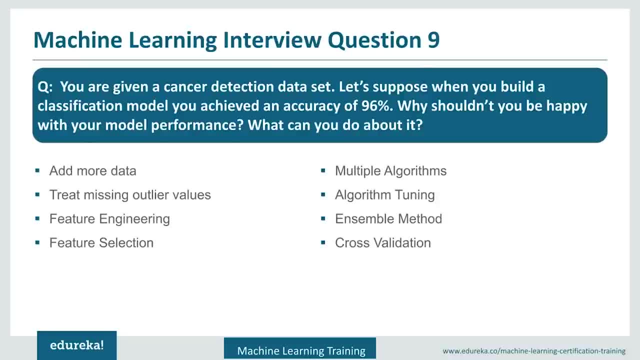 when you build a classification model. you achieved an accuracy of 96%. Why shouldn't you be happy with your model performance? What can you do about it? So first thing is- as this thing is mostly related to the domain of cancer detection interviews, trying to gauge you as how. 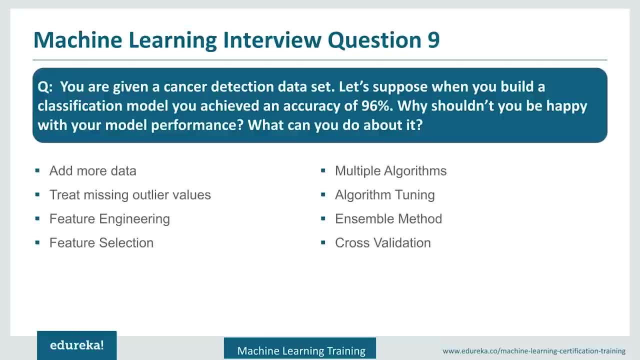 better. you know as so how the accuracy of the models works in a different data distributions. So if we look at the cancer detection domain, in the cancer detection domain very few of your data points would have actual cancer. So, for example, if you have a 1 million patients data, 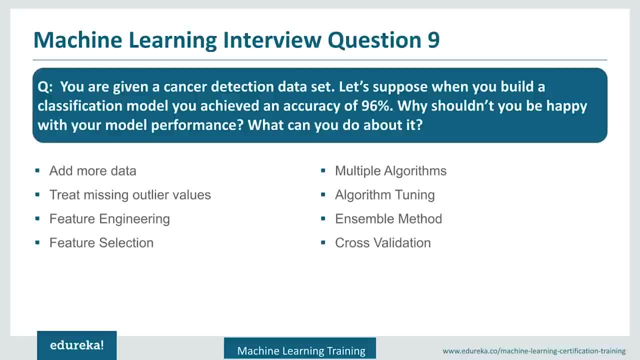 out of that you would have like around 1000 of them would be having cancer, So it's like a very small set of data is having actual cancer. So let's assume we are creating a confusion matrix. So when we create a confusion matrix, 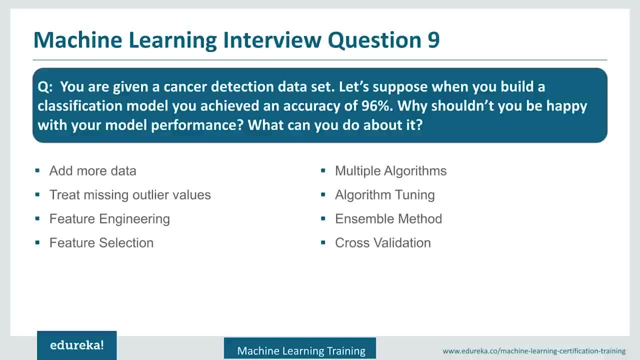 we see that in the true positive, which is just 1000 values. so even if our model tries to identify like 500 of them. so we'll get in the true positive 500 and let's assume in the true negative we are getting all the negative values, which is: 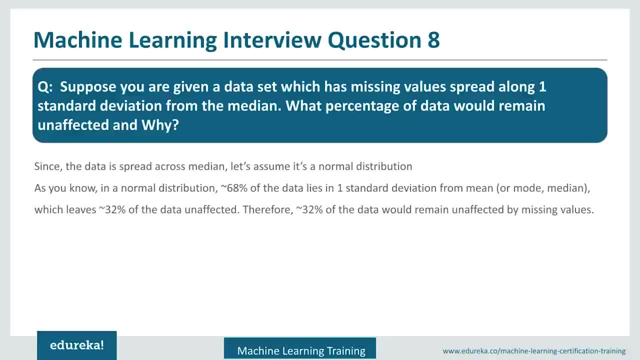 you would assume that this data is also following a normal distribution and you would say that, okay, a normal distribution has, within one standard deviation, a 68 percent of the values. so as per the normal distribution, within one standard deviation around the mean median and mode. as for the normal distribution, all are equal. all mean median mode are at the same location and from the 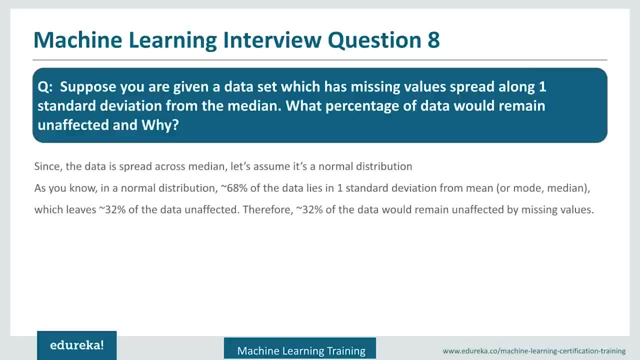 mean around one standard deviation. we would have 68 percent of the values and, as the question says, missing values are spread along one standard deviation. so 68 percent of the values are basically missing and question ask what percentage of data would remain unaffected and why? so everything left after the 68 percent would remain unaffected. so you would say 100 minus 68, that 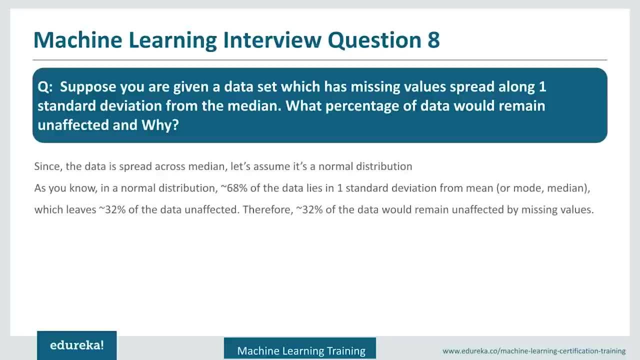 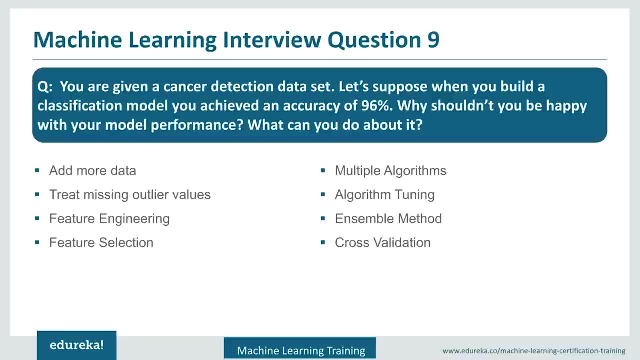 would be 32, so 32 percent of the values would remain unaffected by missing values. you are given a cancer detection data set. let's suppose when you build a classification model you achieved an accuracy of 96. why shouldn't you be happy with your model performance? what can you do about it? 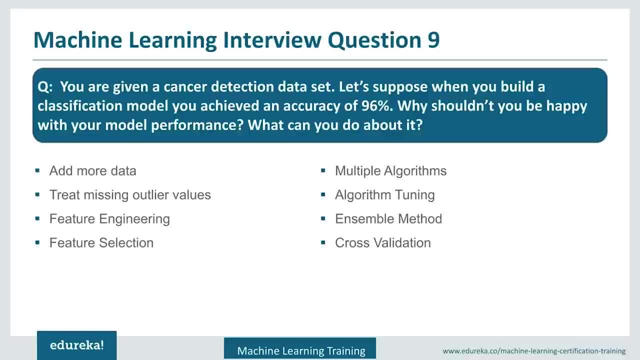 so first thing is, as this thing is mostly related to the domain of cancer detection interviews, trying to gauge you as how better you know, as so how the accuracy of the models works in a different data distributions. so if we look at the cancer detection domain, in the cancer detection domain, very few of your data points would have. 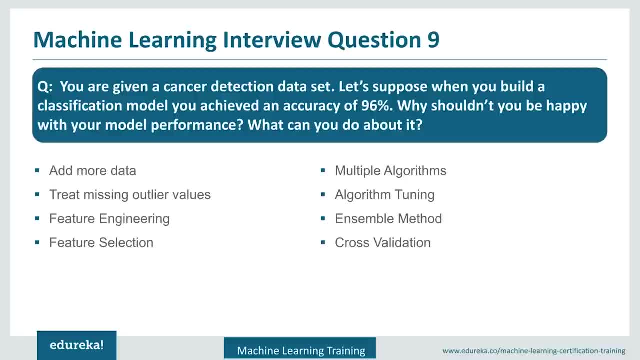 actual cancer. so, for example, if you have a 1 million patients data, out of that you would have like around thousand of them would be having cancer. so it's like a very small set of data is having actual cancer. so let's assume we are creating a confusion matrix. 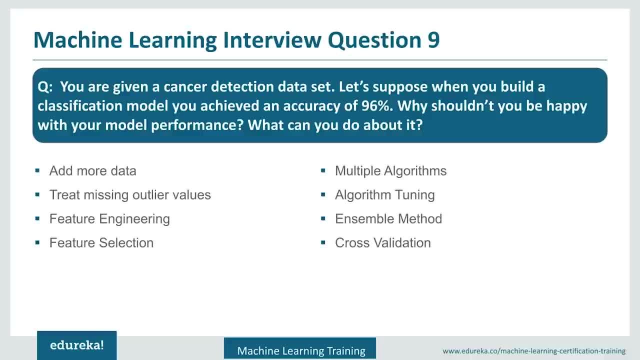 so when we create a confusion matrix, we see that in the true positive, which is just thousand values. so even if our model tries to identify like 500 of them, so we'll get in the true positive 500 and let's assume, in the true negative we are getting all the negative values, which is one. 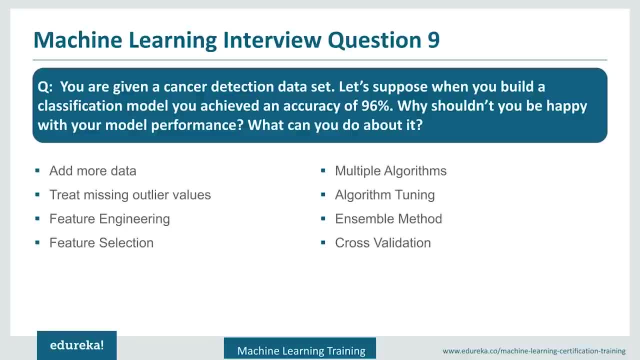 million minus 500, which went into the positives, and everything remaining will go into negative. so if you create the accuracy, it is like 500 divided by whatever is there in the remaining parts. so 500 is what you got: a true positive values and something you will get in the true. 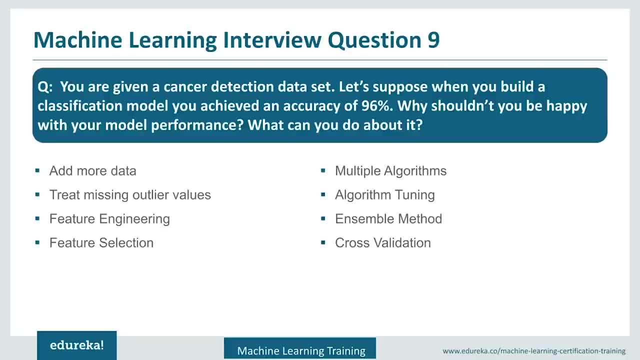 negative and when you divide it you will have a bigger accuracy. so your model give like 98: 96, as your true positive is actually very small, your true negative would be very large and small components will be there in the false positive and false negative. so when you try to 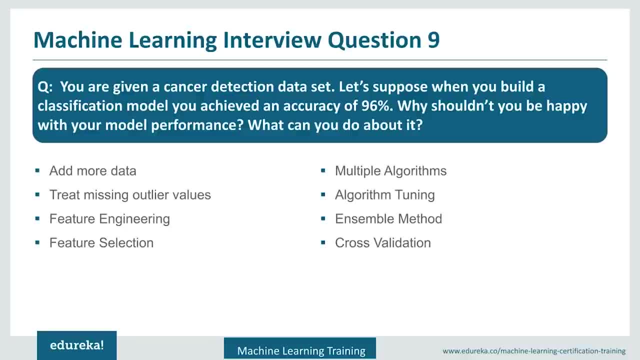 1 million minus 500, which went into the positives, and everything remaining will go into negative. So if you create the accuracy, it is like 500 divide by whatever is there in the remaining parts. So 500 is what you got: a true positive values and 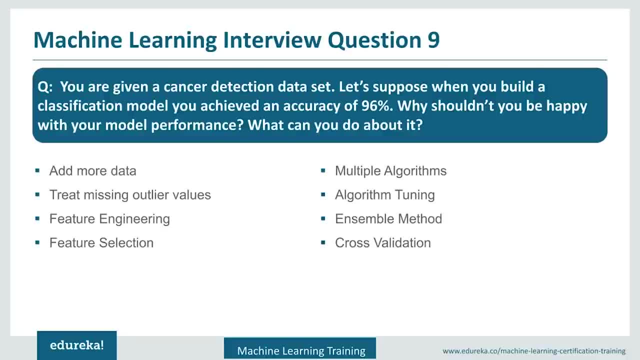 something you will get in the true negative and when you divide it you will have a bigger accuracy. So your model give like 98%- 96%, as your true positive is actually very small. your true negative would be very large and small components will be there in the false positive. 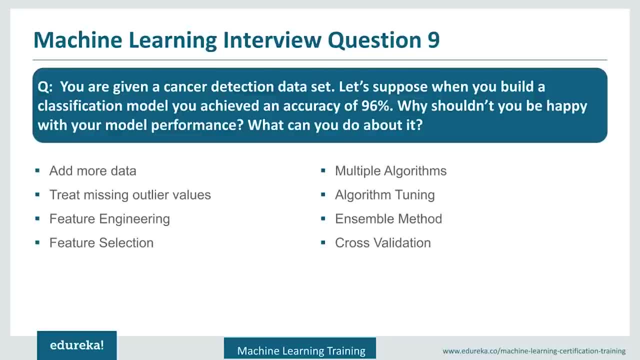 and false, negative. So when you try to divide them you will have a bigger accuracy always. So accuracy is not used in those cases where your distribution of positive cases is very less. So in this case accuracy won't be helpful for us to evaluate the performance. 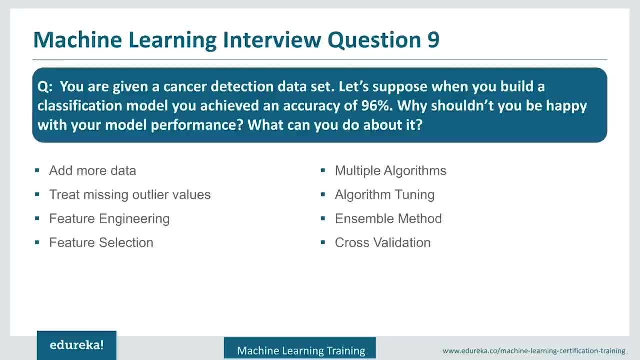 of our model. So we have to go with other performance metrics which are available. So, for example, we have recall, we have precision. recall is again called as the sensitivity. Again we have another as the specificity and F1 score. So this different performance metrics will try to 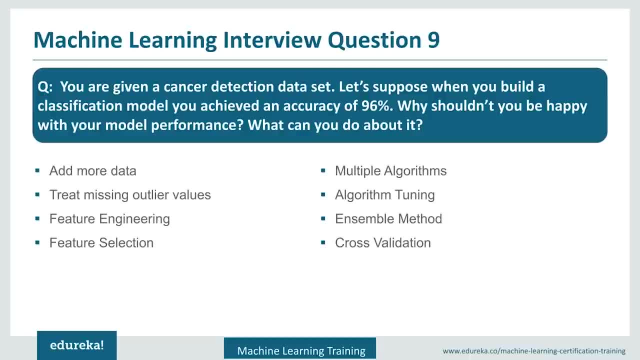 identify the model performance based on different components. So accuracy is mostly useful when you have the classes which have some similar count. When you have some similar count but not very smaller classes, then your accuracy will be helpful. But when you have very small positive class, such as the cancer detection, 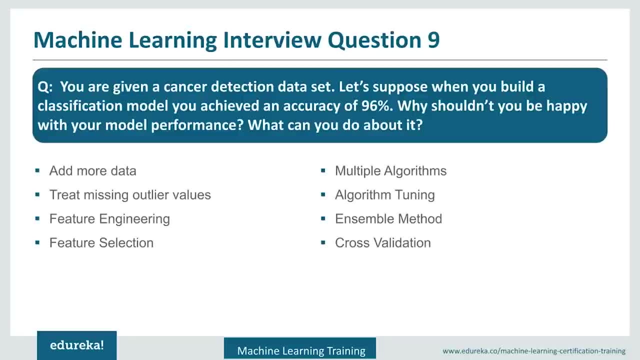 or the anomaly detection. So again, anomaly detection is a similar case where fraud detection basically. So fraud detection is again a case of this case where we have very small number of values. We can't use accuracy in that case and we have to use the different performance metrics. 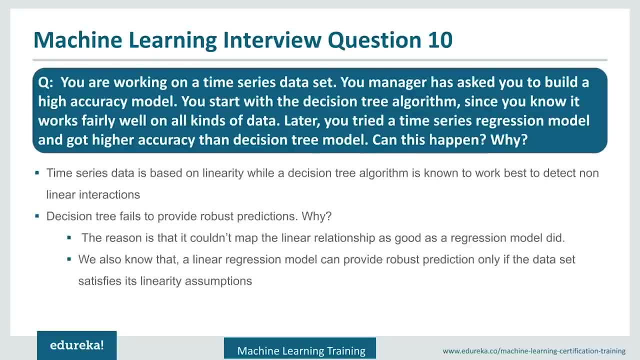 You are working on a time series data set. Your manager has asked you to build a high accuracy model. You start with the decision tree algorithm, since you know it works fairly well on all kinds of data. Later you tried a time series regression model and got higher accuracy. 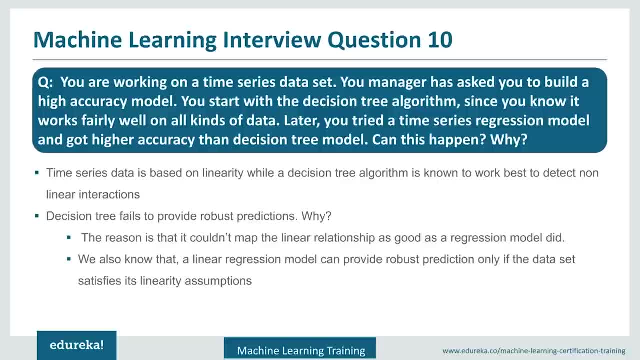 than the decision tree model. Can this happen? Why So? first thing, as it is a time series data. time series data are mostly linear in nature, So as the next value would be related with the previous value, So let's assume we want to look at the stock prices. 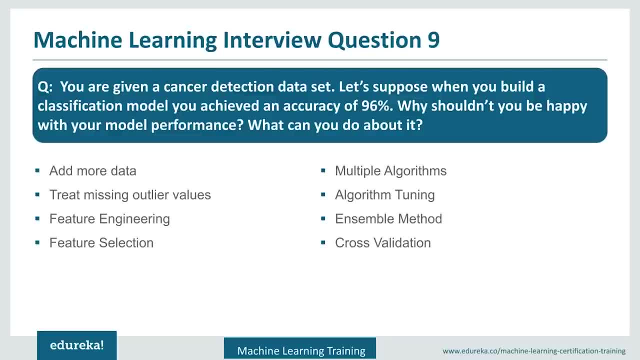 divide them, you will have a bigger accuracy always. so accuracy is not used in those cases where your distribution of positive cases is very less so. in this case, accuracy won't be helpful for us to evaluate the performance of our model, so we have to go with other performance metrics, which are 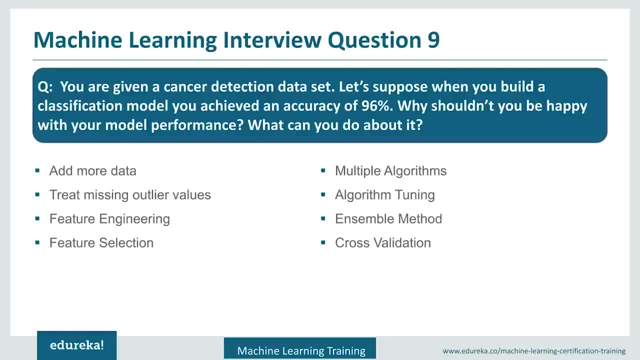 available. so, for example, we have recall, we have precision. recall is again called as the sensitive sensitivity. again we have another as the specificity and f1 score. so this different performance metrics will try to identify the model performance based on different components. so accuracy is mostly useful when you have the classes which have some similar count, when you 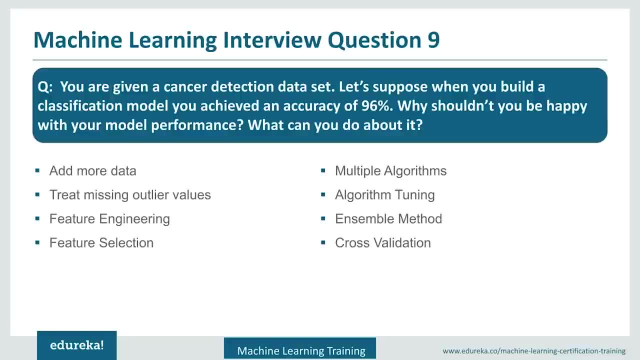 have some similar count, but not very smaller classes, then your accuracy will be helpful. but when you have very small positive class, such as the cancer detection or the anomaly detection, so again Mỹ detection is a similar case where fraud detection basically. so fraud detection is again. 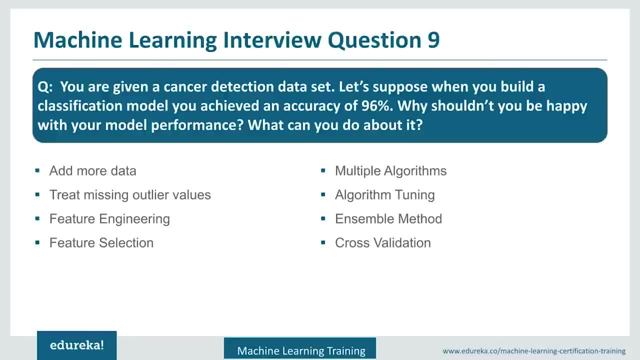 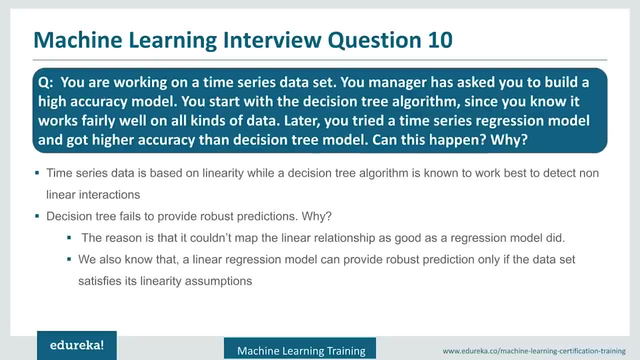 a case of the scale, where we have very small number of values, so we can't use accuracy in that case and we have to use the different performance metrics. you are working on a time series data set. your manager has asked you to build a high accuracy model. 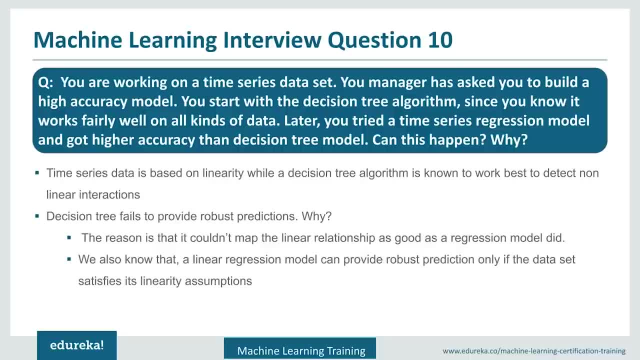 you start with the decision tree algorithm, since you know it works fairly well on all kinds of data. later you tried a time series regression model and got higher accuracy than that time series regression model is on the decision tree model. can this happen? why so? first thing, as it is a time series data. 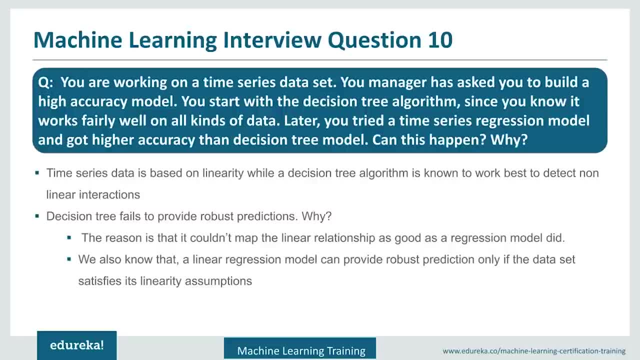 time series data, mostly linear in nature, so as the next value would be related with the previous value, so let's assume we want to look at the stock prices. so stock prices which are today are related with the yesterday. so whatever value was there yesterday, it is the either higher or lower, as 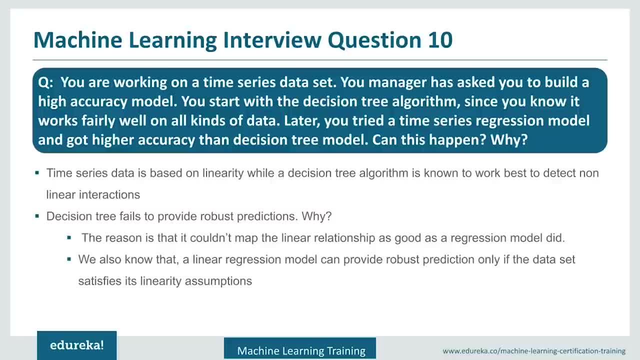 compared to what was there in the yesterday. so, as compared to this, what decision models would do? decision models would just try to identify some rules within your data, so they would just do some rules, which is very non-linear in nature if there is actually some proper patterns within rule. the 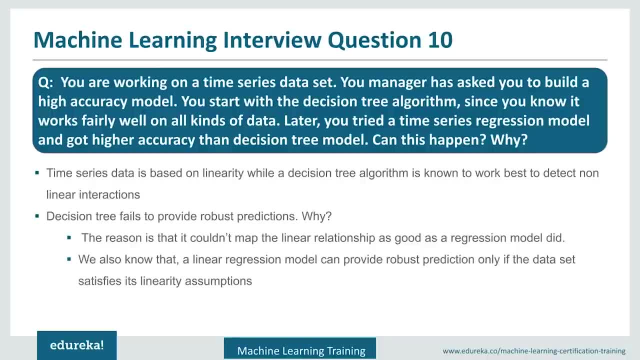 So stock prices, which are today, are related with the yesterday. So whatever value was there yesterday, it is the either higher or lower as compared to what was there in the yesterday. So as compared to this, what decision models would do? decision models would just try to identify. 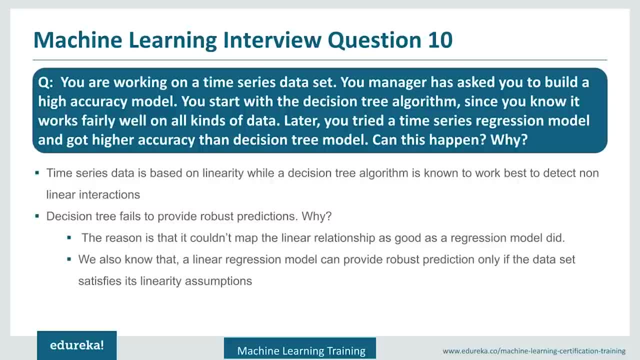 some rules within your data, So they would just do some rules, which is very non-linear in nature. If there is actually some proper patterns within rule, the decision tree would really helpful. But what the time series related regressions would do it? they would try to regress it based on the 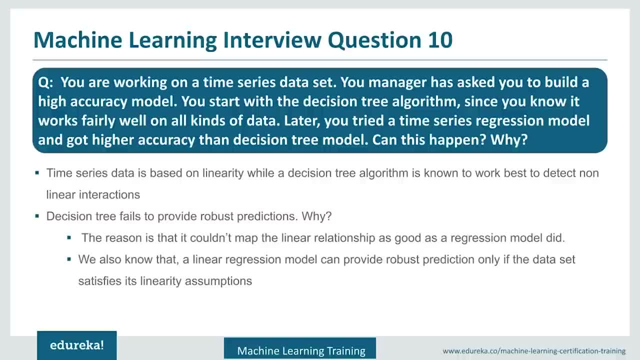 historic value. as they are linearly correlated with the previous values, The time series regressions would work by regressing it on the historic values. So that's why time series regressions would be more accurate than the decision trees, because we have a linearity available. 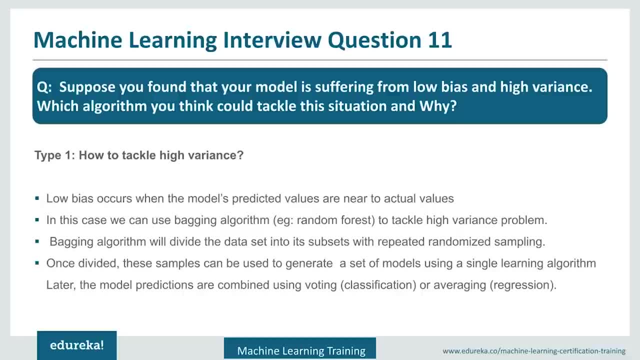 within the time series data. Suppose you found that your model is suffering from low bias and high variance. Which algorithm you think could tackle this situation, and why? So first thing, so low bias and high variance. So bias and variance are the term mostly used. when So bias. 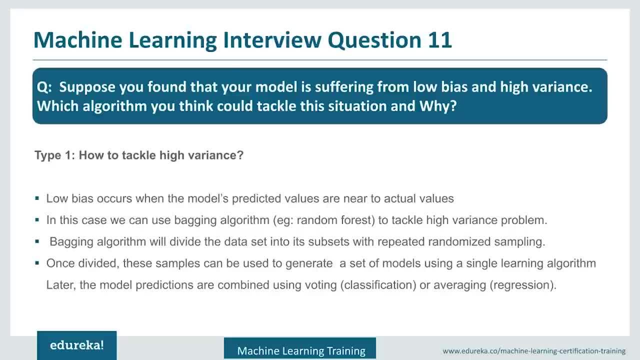 basically means you are getting bias to a specific set. So when you have a higher bias, your model is getting under fit. It's not preferring anything and it is just under fitting your data. And high variance is something where your model is very much over. 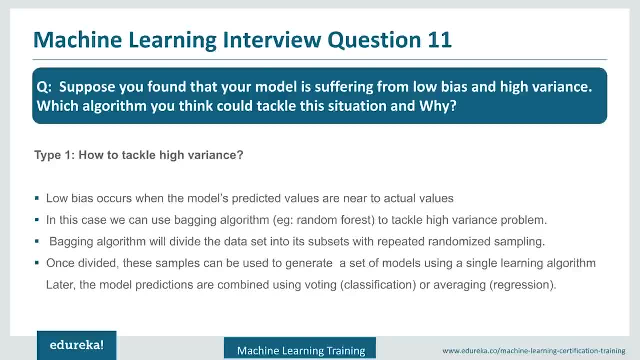 fitting to your data. So in our case it says there is low bias and there is a high variance. So our model is doing a over fit. So first thing is we can use some kind of bagging algorithm. So what, this bagging algorithm? 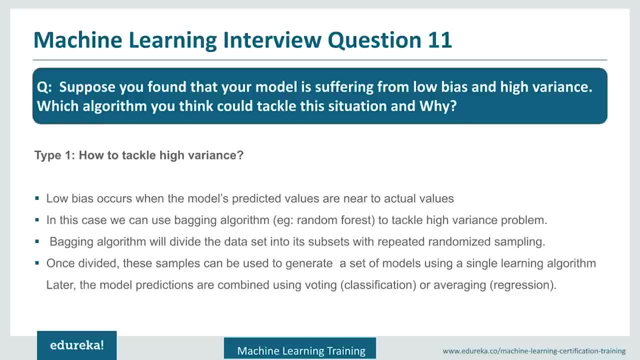 do is they try to divide your data into multiple samples. So those are samples with the replacement, and each sample is trained with the decision tree. So now what happens? we are creating multiple trees which are trying to understand different patterns within the data set. Whatever, 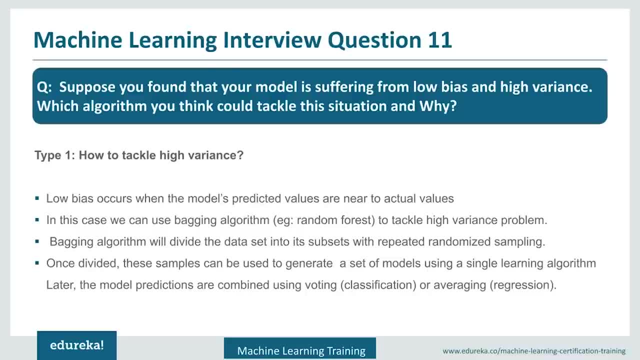 data you are feeding, which your sample you are feeding. whatever the patterns available within that sample, each model is learning those things. So now you have a weak learners and when you combine those weak learners you create a strong learner which will also try to reduce your over fitting. 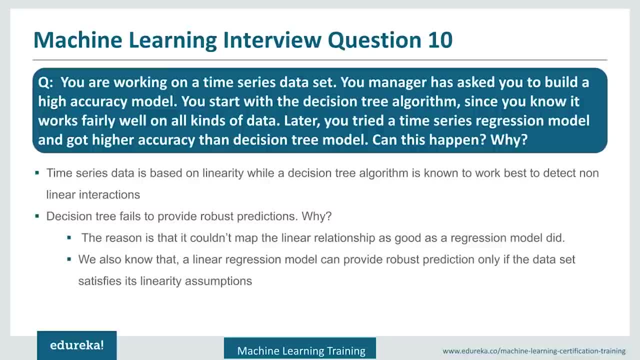 decision tree would really helpful. but what the time series related regression should do it? they would try to regress it based on the historic value, as they are linearly correlated with the previous values. the time series regressions would work by regressing it on the historic values. so that's why time series regressions would be more. 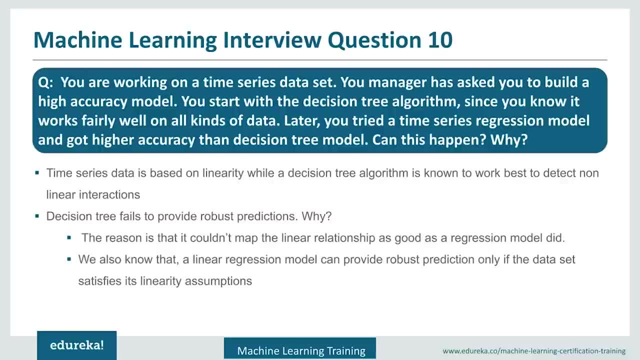 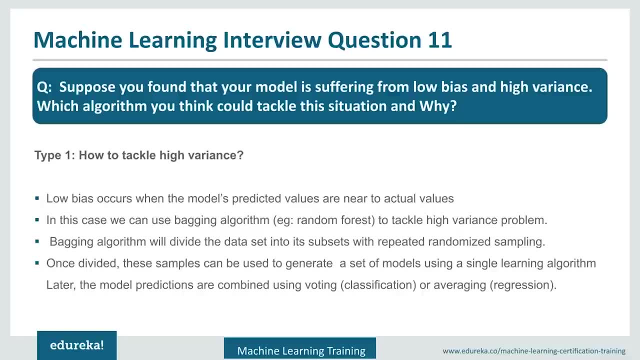 accurate than the decision trees because we have a linearity available within the time series data. suppose you found that your model is suffering from low bias and high variance, which algorithm you think could tackle this situation, and why so? first thing, so low bias and high variance. so bias and variance are the term mostly used when so bias basis. 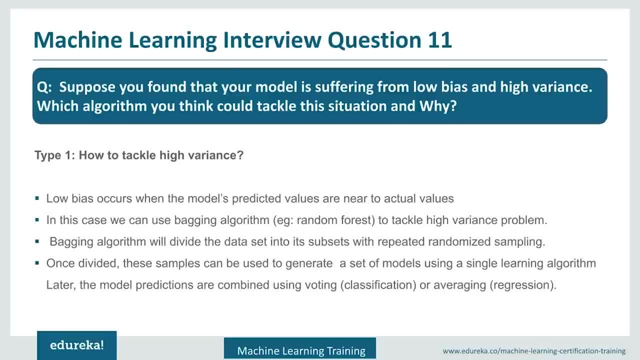 means you're getting biased to a specific set. so when you have a higher bias, your model is getting under fit. it's not preferring anything and it's just under fitting your data. and high variance is something where your model is very much over fitting to your data. so in our case it says there: 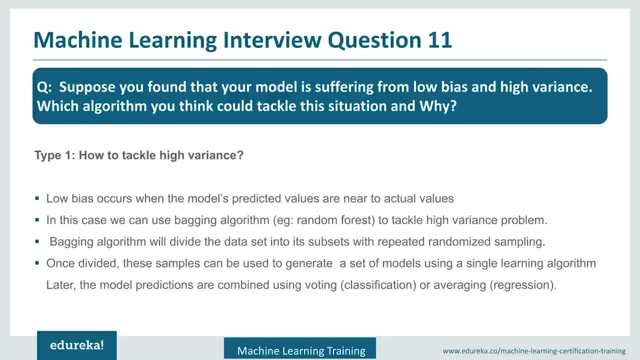 is low bias and there is a high variance, so our model is doing a over fit. so first thing is we can use some kind of bagging algorithms. so what this bagging algorithms do is they try to deal with your data and divide your data into multiple samples. so those are samples with the replacement. 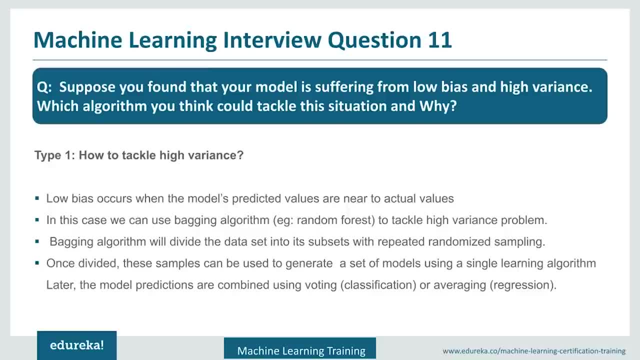 and each sample is trained with the decision tree. so now what happens? we are creating multiple trees which are trying to understand different patterns within the data set. whatever data you are feeding, which your sample you are feeding, whatever the patterns available within that sample, each model is learning those things. so now you have a weak learners. and when you combine those weak learners, 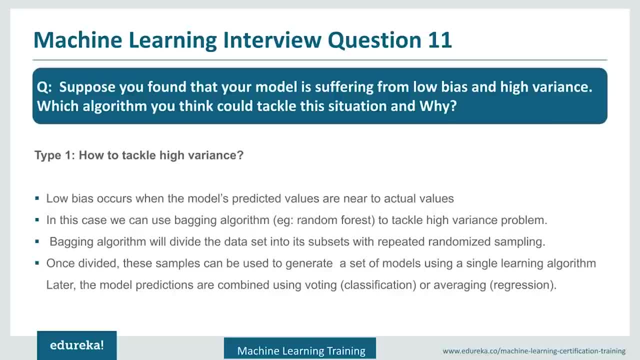 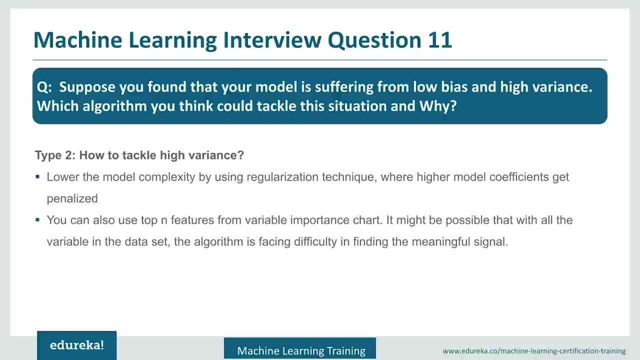 you create a strong learner which will also try to reduce your overfitting. and how it reduces the overfitting is as you're creating more and more models. if some of them is trying to overfit, the others will try to help to get balanced variance. in this case, the other technique that we have is we can use the regularization technique. 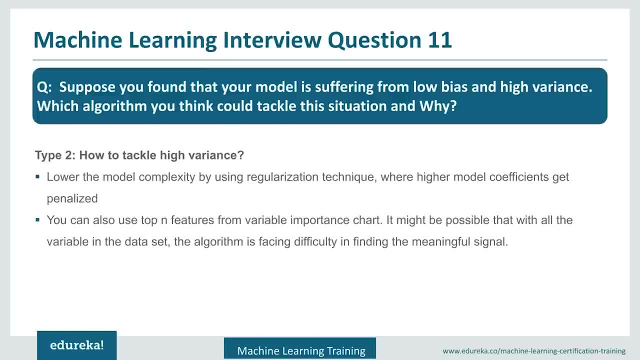 so regularization. there are two types of regularization. there is l1 regularization and there is l2 regularization, those techniques we can use to penalize the model. so what happens? those try to penalize whenever your model goes for a higher variance, it tries to penalize it by some parameters that we provided. so, based on those parameters, it tries to restrict. 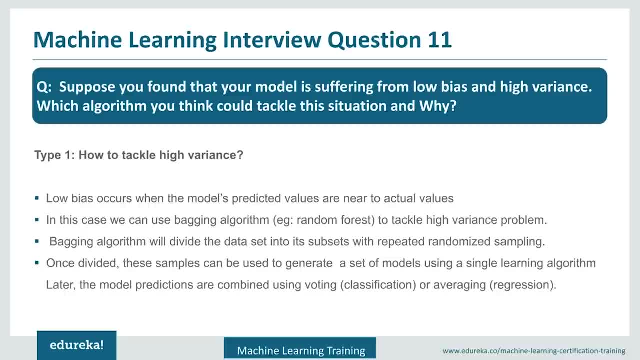 and how it reduces the over fitting is. as you are creating more and more models. if some of them is trying to over fit, the others will try to help to get balanced variance. in this case, The other technique that we have is we can use the regularization technique. So regularization. 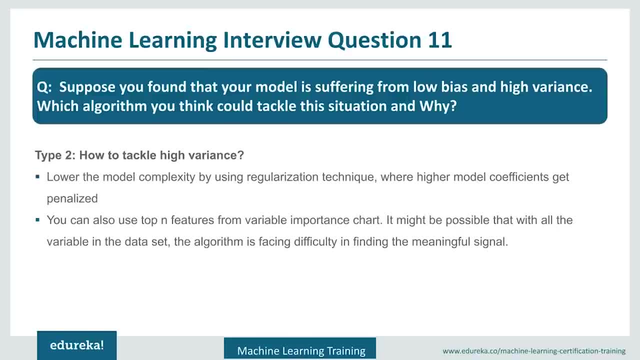 there are two types of regularization. There is L1 regularization and there is L2 regularization- Those techniques we can use to penalize the model. So what happens? those try to penalize. whenever your model goes for a higher variance, it tries to penalize it by some. 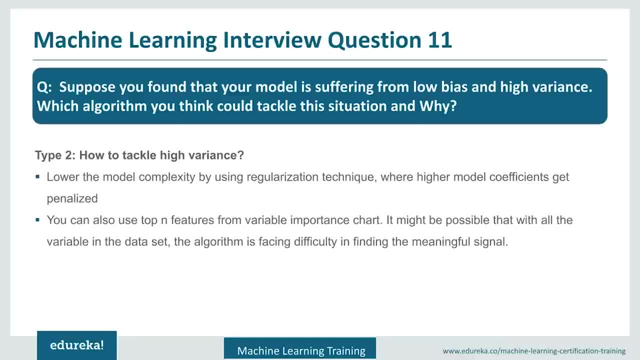 parameters that we provided. So based on those parameters, it tries to restrict your model for going beyond the limited threshold of the over fitting. So the regularization is the second technique. and third is we can use the feature importance. So we can use the different tree based techniques like we can. 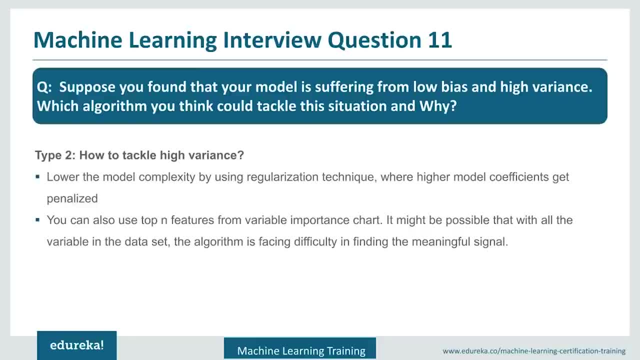 use the random forest, like feature importance techniques, to select top features and we can use those to create a model so that our model will try to fit with those important features. So when we try to add all the features, some features may make our model very much over fitted. and when we 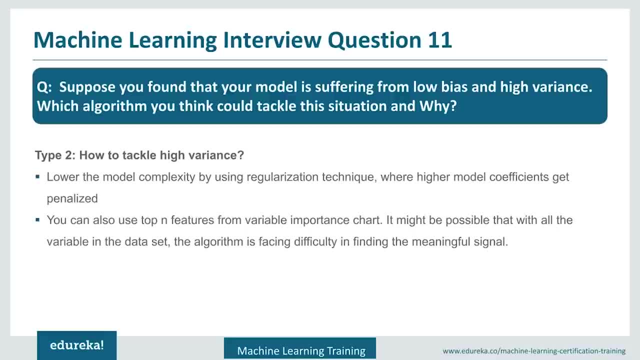 have a newer data, it may not generalize well. So when we try to identify which are the important features, then our model will try to generalize well to the actual patterns which are there within the data. So it's always better to go with feature importance. try to select the features which are important. 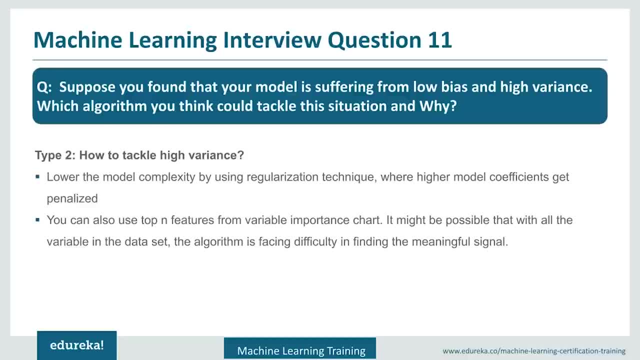 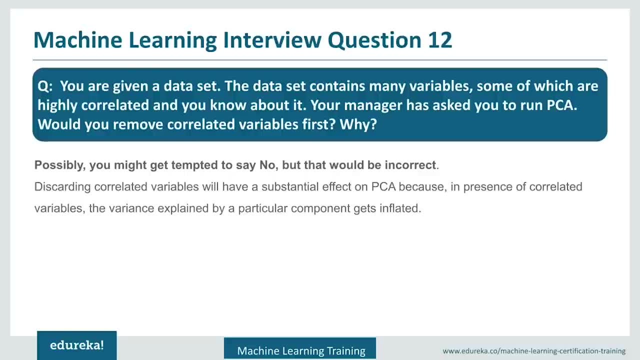 then create our model on top of it. So these are the three techniques that we can use to reduce the variance. You are given a dataset. the dataset contains many variables, some of which are highly correlated, and you know about it. Your manager has asked you to run PCA, Could you? 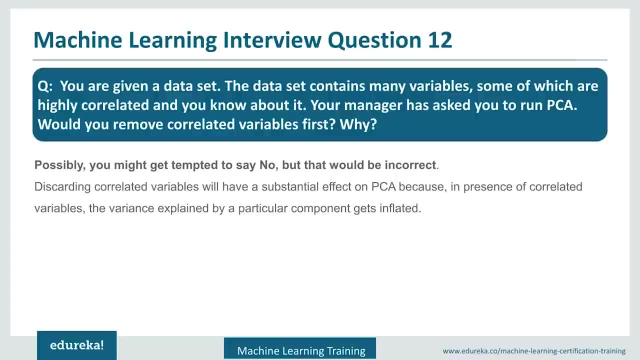 remove correlated variables first, and why So? most of the people would say that okay, PCA we are using to reduce the multicollinearity. so, removing the collinear variables, we won't use the PCA. But what happens is we are with the PCA, we are not just interested with the 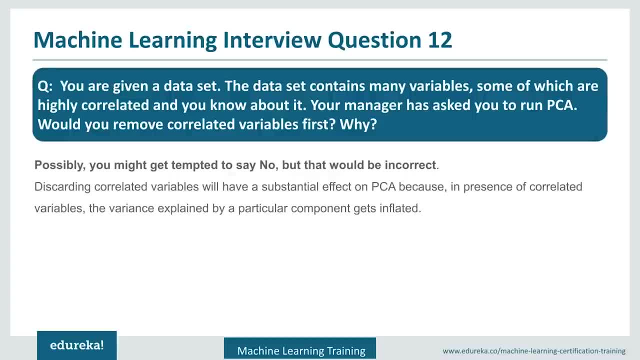 multicollinearity of the variables. Sometimes we are also interested with the variance which is available within the data. So what happens is PCA tries to explain a complete variance available within your data. So variance is something which says like the distributions within your data. So once you know that, 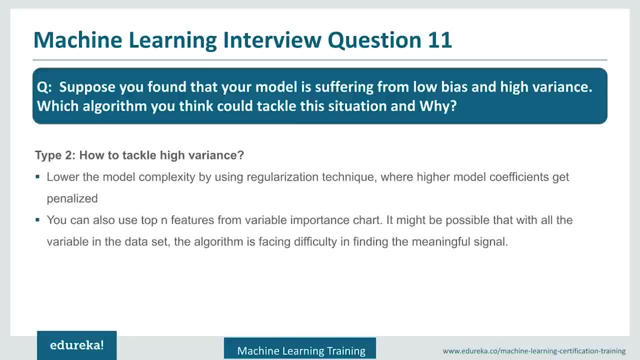 your model for going beyond the limited threshold of the overfitting. so the regularization is the second technique. and third is we can use the feature importance so we can use the different tree based techniques, like we can use the random forest, like feature importance techniques to select top features and we can use those to create a model so that our model will try to 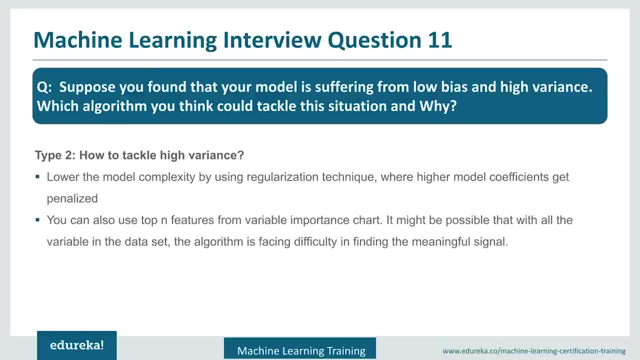 those important features. so when we try to add all the features, some features may make our model very much overfitted and when we have a newer data it may not generalize well. so when we try to identify which are the important features, then our model will try to generalize well to the actual 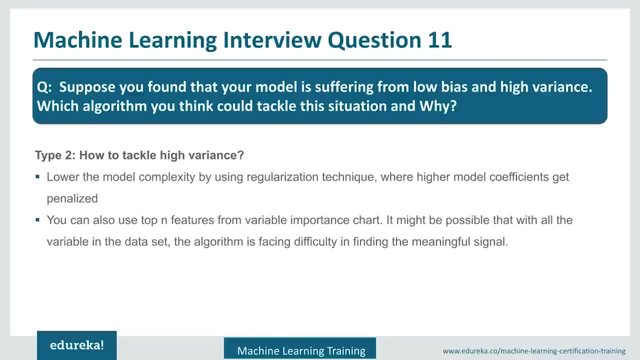 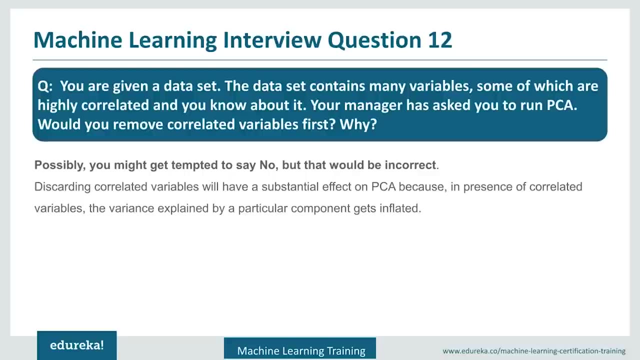 patterns which are there within the data. so it's always better to go with feature importance. try to select the features which are important, then create our model on top of it. so these are the three techniques that we can use to reduce the variance. you are given a data set. the data set contains many variables, some of which are highly correlated. 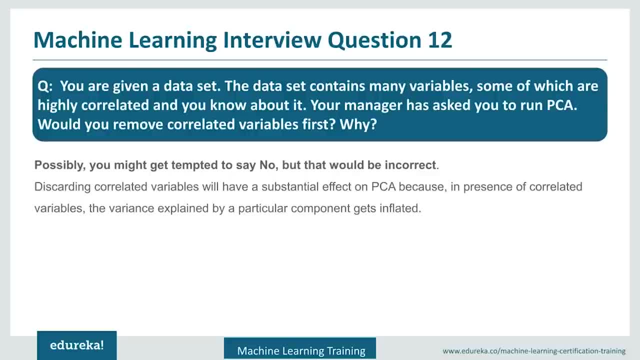 and you know about it. your manager has asked you to run pca. would you remove correlated variable first? and why so? most of the people would say that okay, pca we are using to reduce the multicollinearity. so, removing the collinear variables, we won't use the pca. but what happens is we are with the pca. we 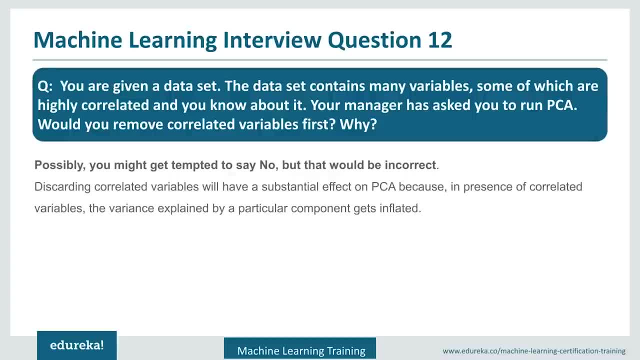 are not just interested with the multicollinearity of the variables. sometimes we are also interested with the variance which is available within the data. so what happens is pca tries to explain a complete variance available within your data. so variance is something which saves, like the distributions within your data. so once you know that, pc also gives you the eigen. 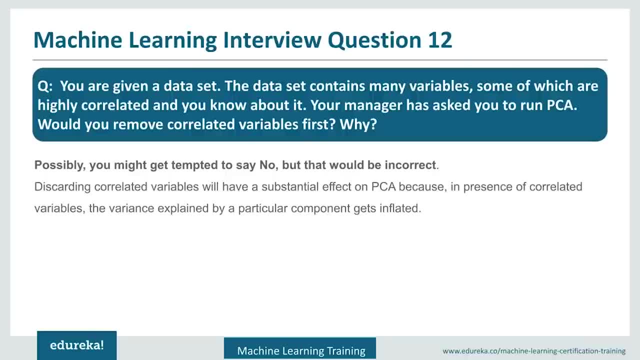 vector through this variance and you can use this variance to reduce the features which are available to you. even when there is no multicollinearity, even if you have some thousand features, there is no linearity within the variables. When you use the PCA in, still, in this case also, you will be able. 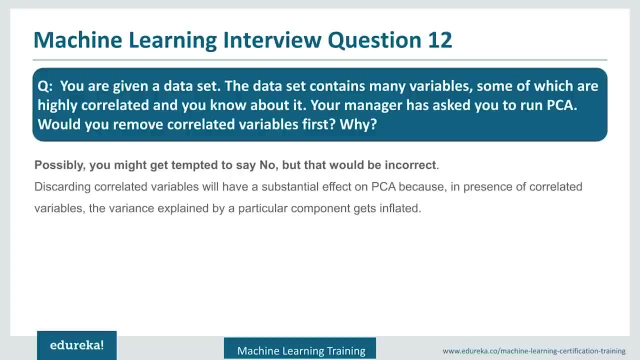 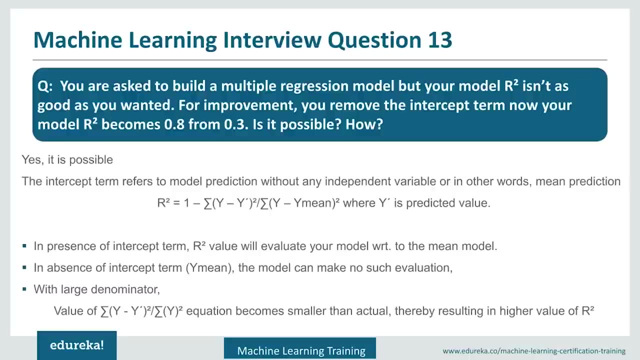 to reduce the size of your features to a lesser number. So PCA doesn't just has to be with the correlated variables, We can use it also just to reduce the columns length using the variances which are explained in the model. So you are asked to build a multiple regression model, but your 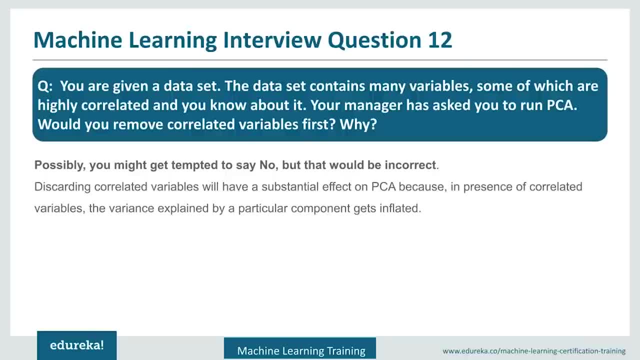 PCA also gives you the eigenvector through this variance and you can use this variance to reduce the features which are available to you, even when there is no multicollinearity. Even if you have some thousand features, there is no collinearity within the 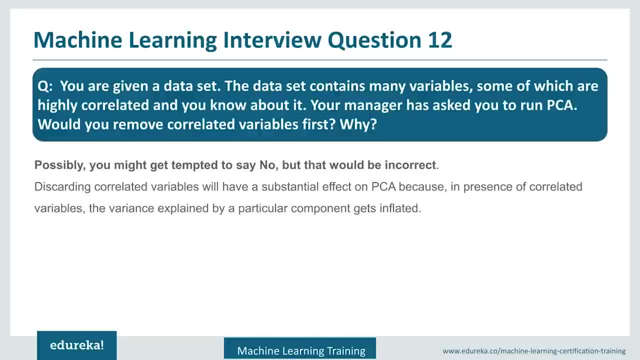 variables. When you use the PCA- and still in this case also, you will be able to reduce the size of your features to a lesser number. So PCA doesn't just has to be with the correlated variables, We can use it also just to reduce the columns. 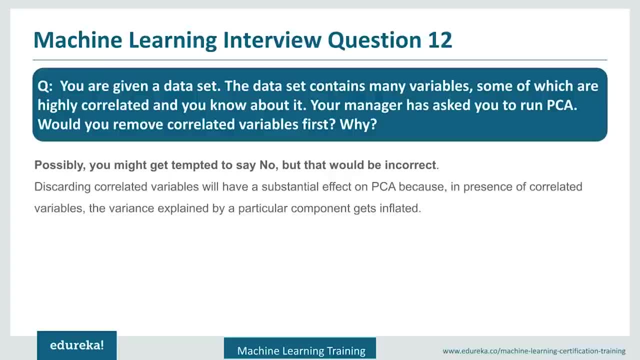 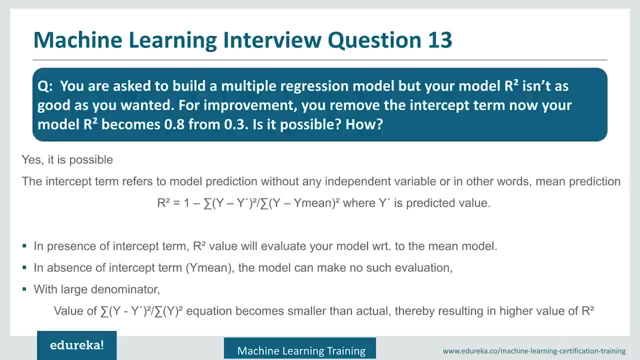 length using the variances which are explained in the model. So you are asked to build a multiple regression model, but your model R square isn't as good as you wanted. For improvement, you remove the intercept term. now your model R square becomes 0.8. 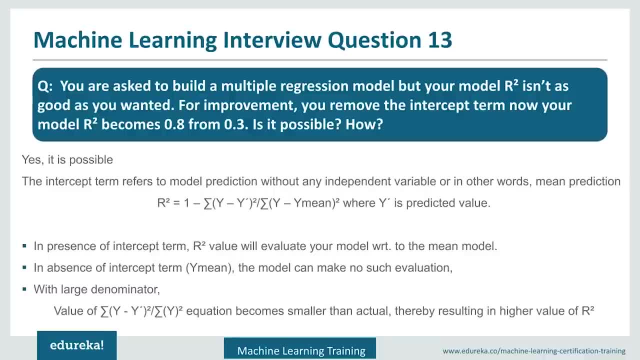 from 0.3.. Is it possible and how? So, first thing, what is R square? So R square says how your linear regression model, how much of the variance out of the data it's trying to explain. So your data contains a variance and 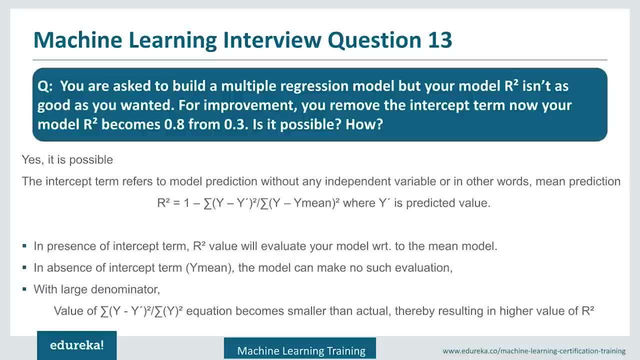 what percentage of variance your model is trying to explain. The more the variance it is trying to explain, the better is your model trying to represent your data. So the formula if we see for the R square is: R square is equal to 1 minus summation of. 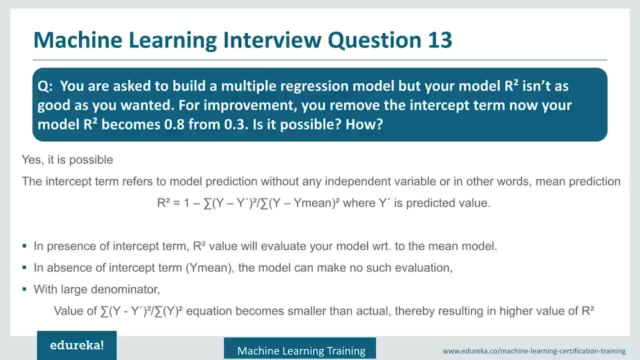 y minus y hat, which is the predicted values square upon y minus y mean square. So intercept basically refers to the y mean. So in actual, the intercepts are representing the y mean and they are helping the model to maintain based on the y mean. So in the presence. 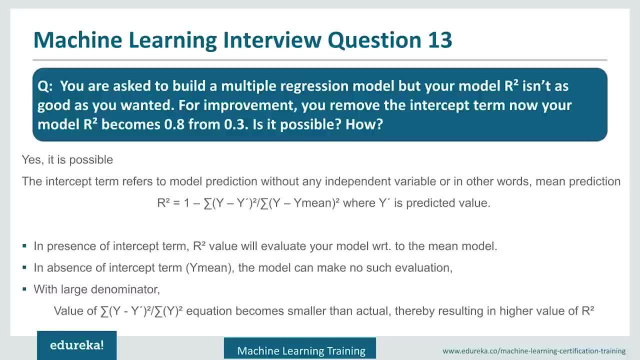 of it, we are creating R square, which is something different, and when we are removing the y mean, so when we are removing the intercept, we are removing the y mean. in our case, as a denominator becomes small, R square would become big. So, as we remove the y mean, our denominator, 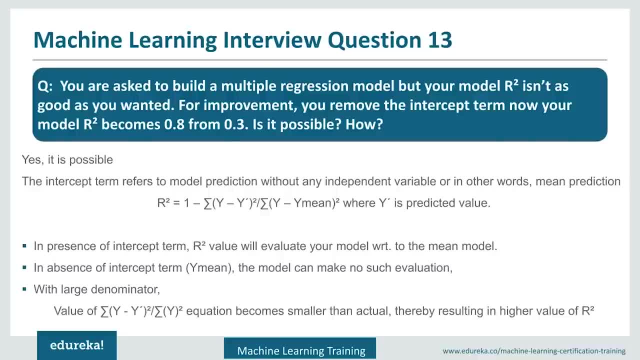 would become small and, as we are dividing by that, our R square would become big. But one thing that you have to be very sure in this case is this: both the models are different. You cannot compare the model without the intercept and the model with the intercept. So 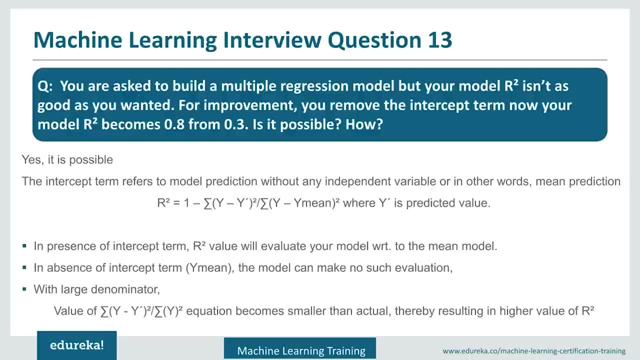 model R square isn't as good as you wanted For improvement. you remove the intercept term. Now your model R square becomes 0.8 from 0.3.. Is it possible and how? So, first thing, what is R square? So R square says how your linear regression model how much of the variance out of the data it's. 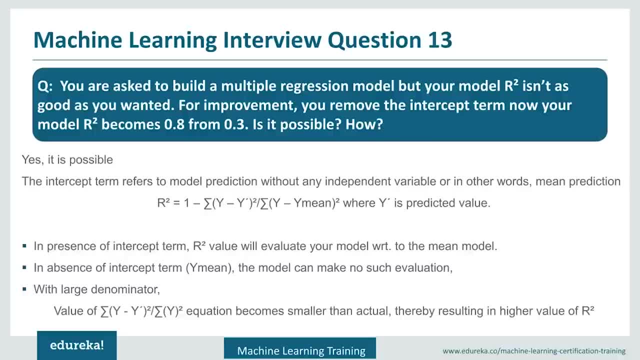 trying to explain. So your data contains a variance and what percentage of variance your model is trying to explain. The more the variance it is trying to explain, the better is your model trying to represent your data. So the formula, if we see for the R square is: R square is equal to 1 minus summation of Y minus Y hat, which is the 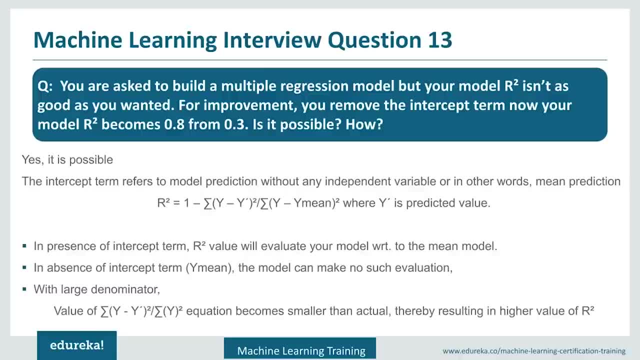 predicted values square upon Y minus Y mean square. So intercept basically refers to the Y mean. So in actual, the intercepts are representing the Y mean and they're helping the model to maintain based on the Y mean. So in the presence of it, we are creating R square, which is something different. 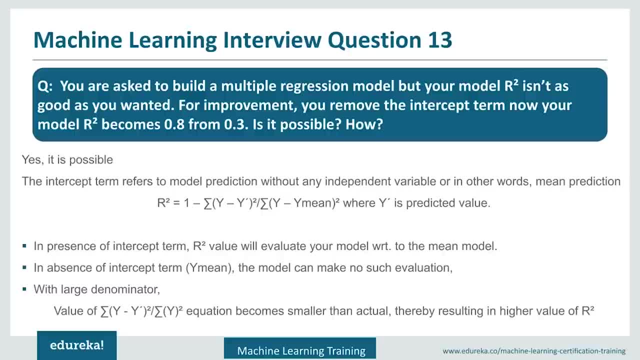 when the Y a. removing the Y means When we are removing the intersect, we are the learning. the Y mean, in our case, As a denominator becomes small, R square is I 임 come back. So as we remove the Y mean are denominator would become small And I'm there dividing by that, R squared would become big. But one thing: 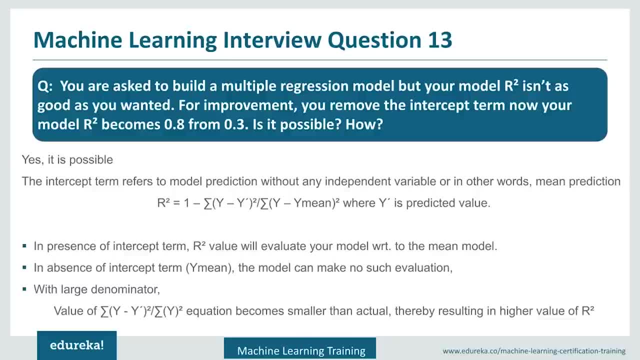 that you have to be very sure in this case is that both these models are different. You cannot compare the model without the intercept. I'm the model with the intercept. So this: both the models are different And you to tune them separately and you have to measure them separately. they cannot be compared as the. 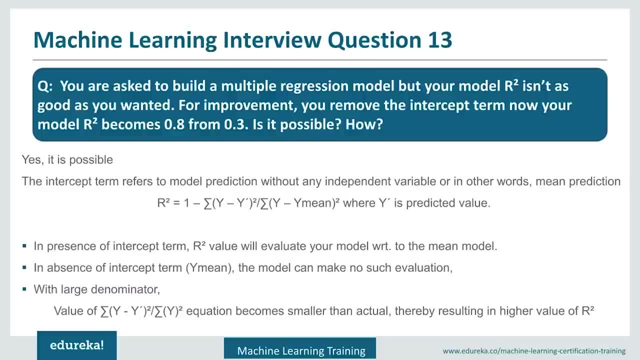 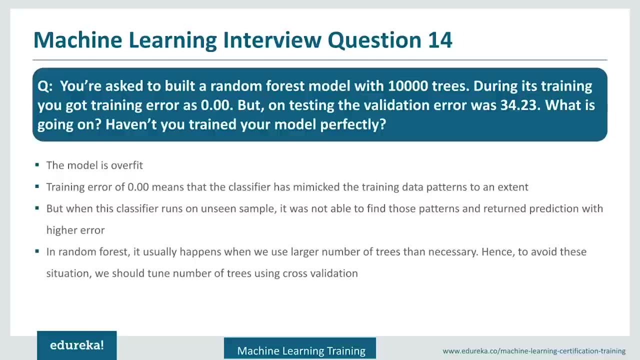 one with the intercept and without the interceptor, completely different in nature. you are asked to build a random forest model with 10 000 trees. so during its training, you got training error 0.0, but on testing the validation error was 34.23. what is going on in this case? haven't you trained your? 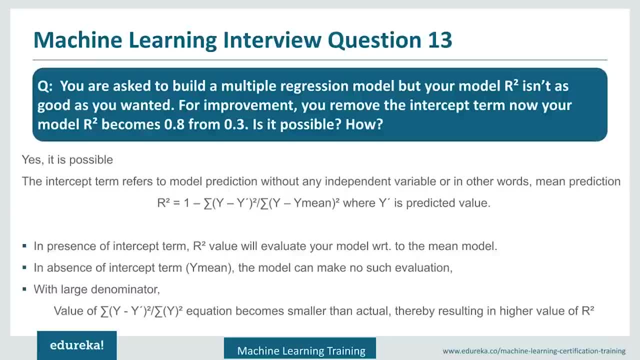 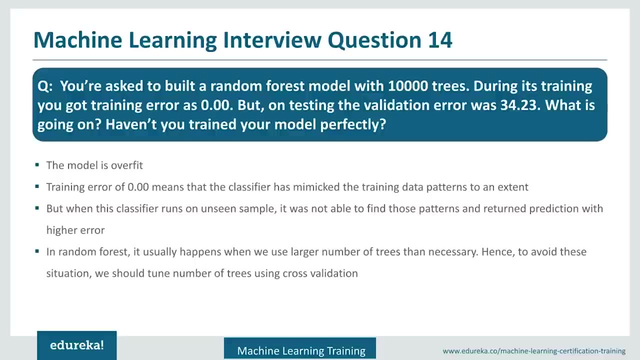 both the models are different and you have to tune them separately and you have to measure them separately. They cannot be compared as the one with the intercept and without the intercept are completely different in nature. You are asked to build a random forest model with 10,000 trees. So during 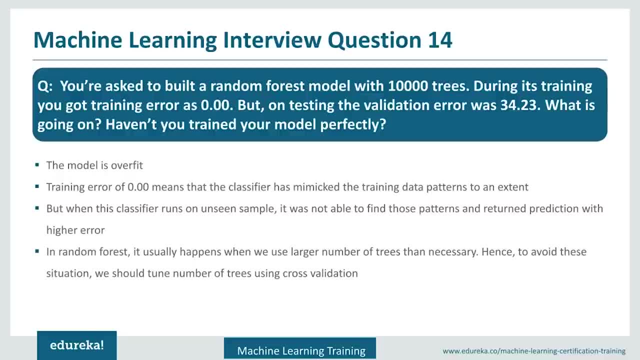 its training. you got training error 0.0, but on testing the validation error was 34.23.. What is going on in this case? Haven't you trained your model perfectly? So this was very good. that right got a 0.00 like. 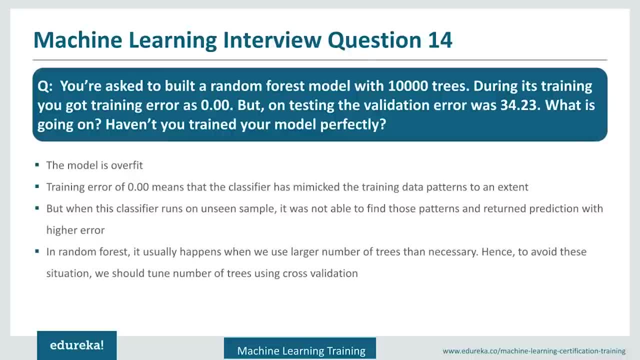 100% accuracy with the training data, But when we try on the validation dataset, we say that it is there is an error of 34.23 of some metric, For this case basically says is: you are getting very much good performance on the training data, but when you check it on the 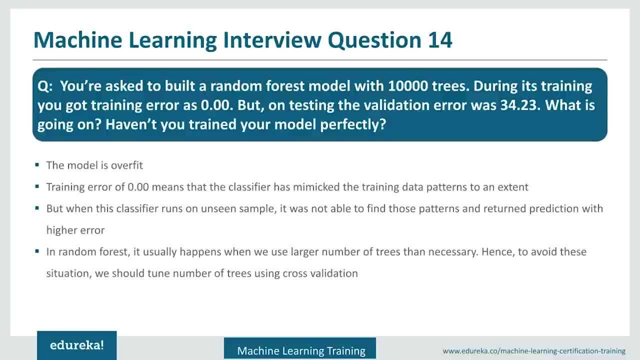 unseen data. this unseen data is showing some different performance. So this is an pure example of complete over fitting. So what you are doing is your model is trying to learn mimic actual data within the training set. It is just learning every pattern, every corner of your 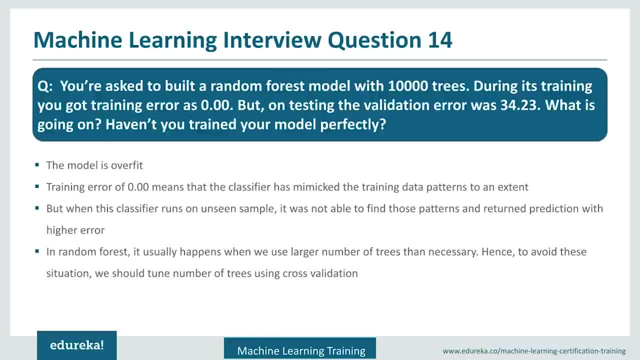 data and it is trying to make actual and accurate predictions out of it. But when we go for a new data, as it has got very much mimicking the training data, so newer data may get the outer bounds and may not get a better predictions. So we have to reduce. 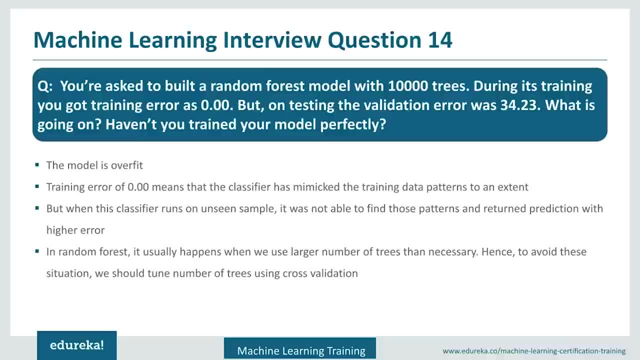 the over fitting and try to make a model, generalize. So we can use these things that we have discussed earlier to reduce the over fitting within the data. So we can use different techniques that we already discussed, such as we can provide more data or we can reduce. 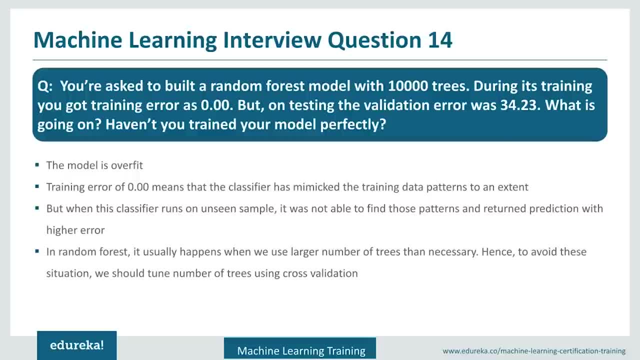 the number of trees which are there. So as we are using more and more trees, our model is getting over, fitted to the data. So in our case we have to use the lesser number of trees and see if our model gets generalized or not. So, people, 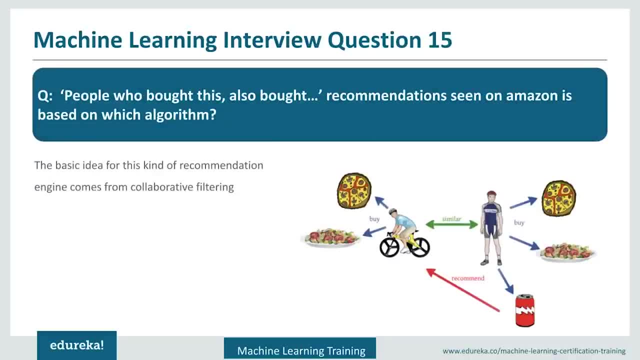 who brought this also brought recommendation seen on Amazon is based on which algorithm. So we have all seen on Amazon that when we are looking at some product, we get that. okay, people have also brought this kind of product. What basically this means is: whatever you are currently looking, 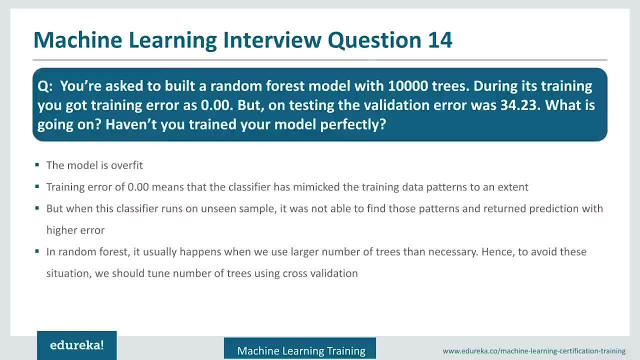 model perfectly. so this was very good. that right got a 0.00 like 100 accuracy with the training data, but when we try on the validation data set, we say that it is there is an error of 34.23 of some metric. what this case basically says is: you are getting very much good performance on the. 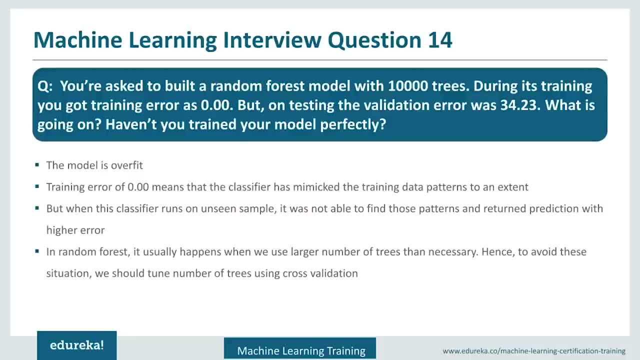 training data, but when you check it on the unseen data, this unseen data is showing some different performance. so this is an pure example of complete over fitting. so what you are doing is your model is trying to learn mimic actual data within the training set. it is just learning every pattern, every corner of your data and it's trying to make 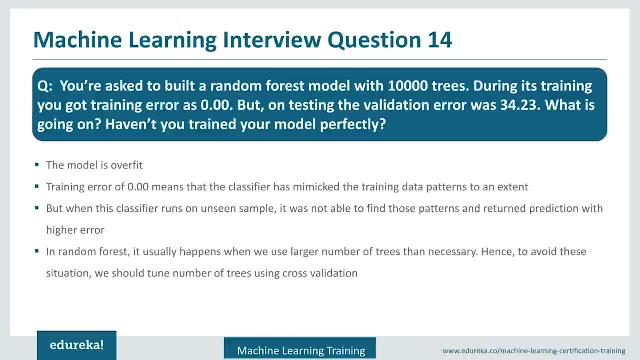 actual and accurate predictions out of it. but when we go for a newer data, as it has got very much mimicking the training data, so newer data may get the outer bounds and may not get a better predictions. so we have to reduce the over fitting and try to make a model. 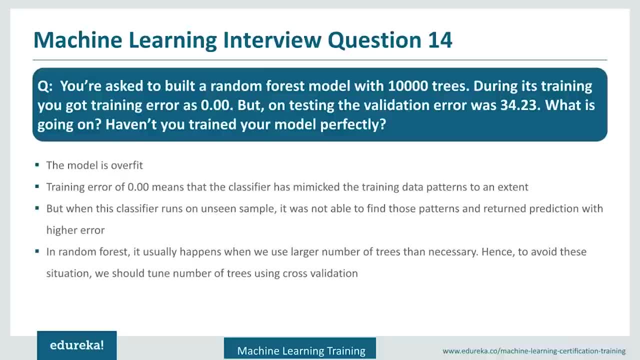 generalize. so we can use these things that we have discussed earlier to reduce the over fitting within the data. so we can use different techniques that we've already discussed, such as we can provide more data or we can reduce the number of trees which are there, so as we are using more and 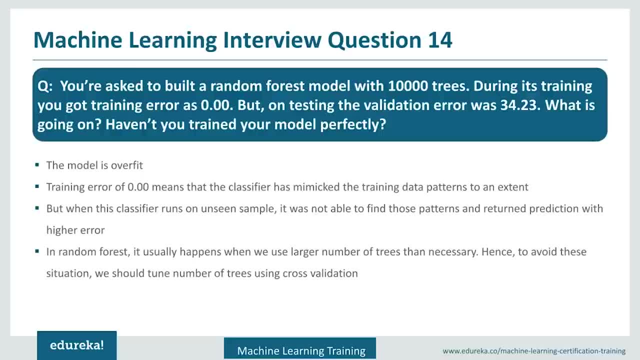 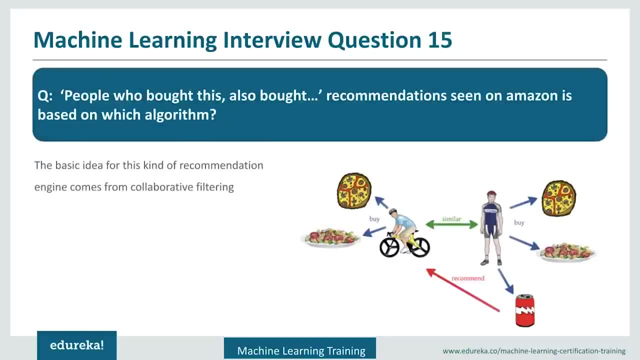 more trees. our model is getting over fitted to the data, so in our case we have to use the lesser number of trees and see if our model gets generalized or not. so people who brought this also brought recommendation. recommendation seen on amazon is based on which algorithm? so we have all seen on amazon that when 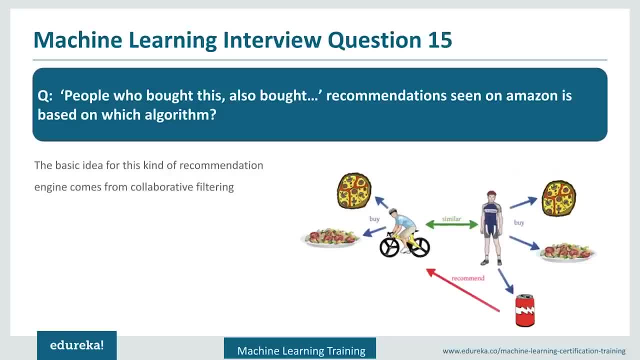 we are looking at some product, we get that. okay, people have also brought this kind of product. what basically this means is: whatever you are currently looking, people who have brought that product or who have already viewed that product have also looked at the different products. so, based on those, you are getting recommendations. so there are two types of recommendation systems. 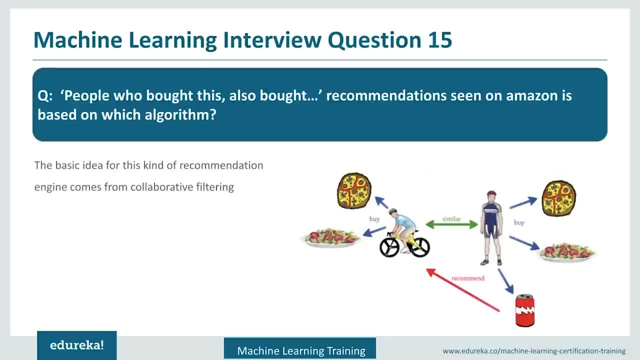 first is the collaborative filtering and second is the content-based filtering. in content-based filtering, what happens is whatever you have rated previously, so based on that, you will get a future recommendation. so, for example, let's take an example of netflix. in netflix, you have watched some genre movie you have watched. 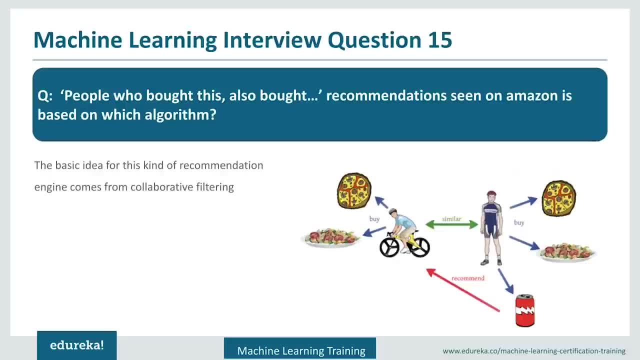 people who have brought that product or who have already viewed that product have also looked at the different products. So based on those you are getting recommendations. So there are two types of recommendation systems. First is the collaborative filtering and second is the content based filtering In content. 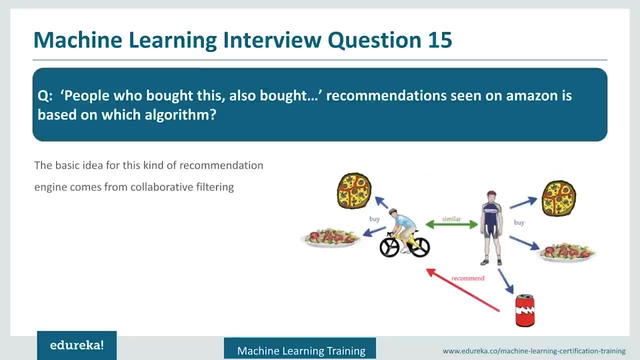 based filtering. what happens is whatever you have rated previously, based on that, you will get a future recommendation. So, for example, let's take an example of Netflix. In Netflix, you have watched some genre movie. You have watched romantic movie for two to three times and you have given a better rating. 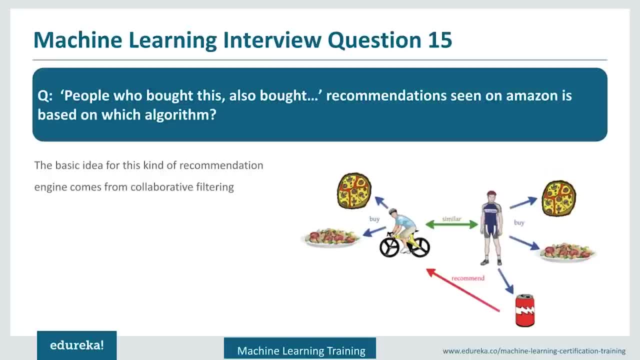 So what Netflix would do: based on whatever you have done, whatever the content we have viewed earlier, it will create a new recommendation for you. So, based on whatever you have done previously, you will get a newer recommendation. So that is the content based recommendation. What we 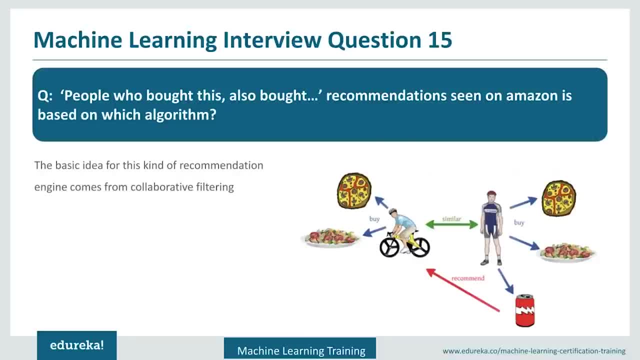 are seeing currently for this example, it is collaborative filtering. In collaborative filtering, what happens is whatever you are doing or whatever you have done previously. based on that, you will be checked with the other users who have done similar activity and it will also check what are all different activities they have done. 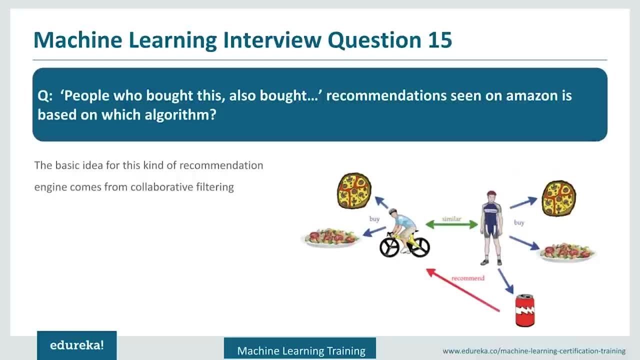 and you have not done that, It will try to recommend those things to you. So if you see the example which is here, it says that the user who is on bicycle has brought pizza and pasta. Similarly, he is trying to be compared with the user who has done. 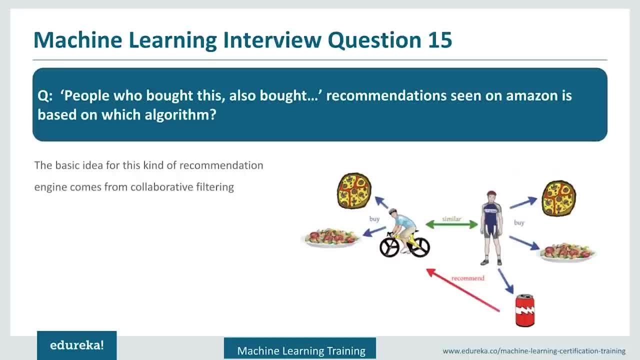 similar activity. So in our case, there is this user who has brought pizza, pasta plus a coke. So as the user has not brought coke, he will be recommended this coke. So this is the core of collaborative filtering. So this is the technique which all the major e-commerce 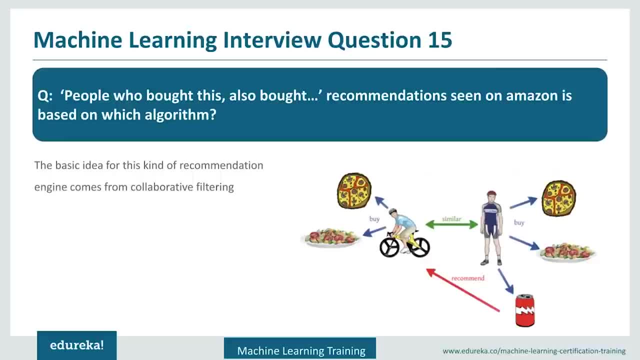 related companies use to recommend products to the users. So even Netflix just uses the content based filtering for recommending the products based on the history that he has done. But also he will be recommended based on the collaborative filtering as what all other users have done similarly and what they have done. 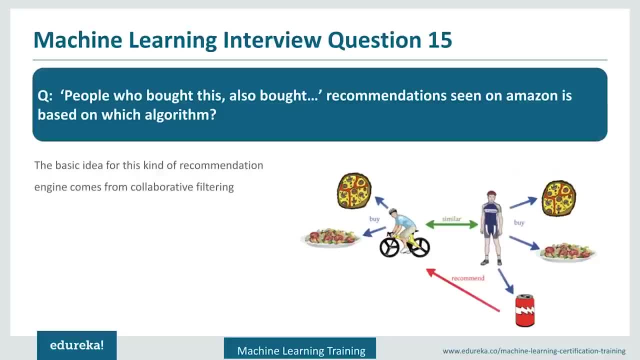 as additional things. So that's how the recommendation system works, Just to summarize what we have done today. So basically, we have started with the three components, three types of interview questions. We started with the core machine learning components, which involved more of a theoretical components. 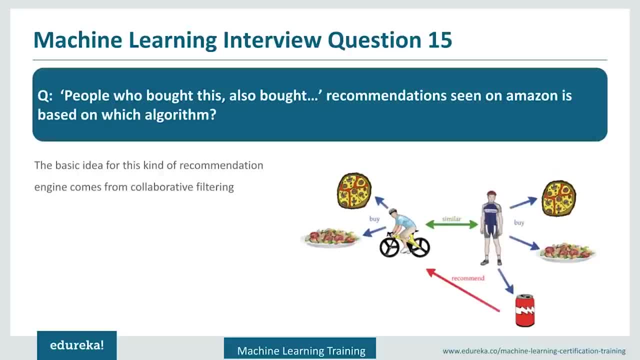 romantic movie for two to three times and you have given a better rating. so what netflix would do? based on whatever you have done, whatever the content we have viewed earlier, it will create a new recommendation for you. so, based on whatever you have done previously, you will get a newer recommendations. 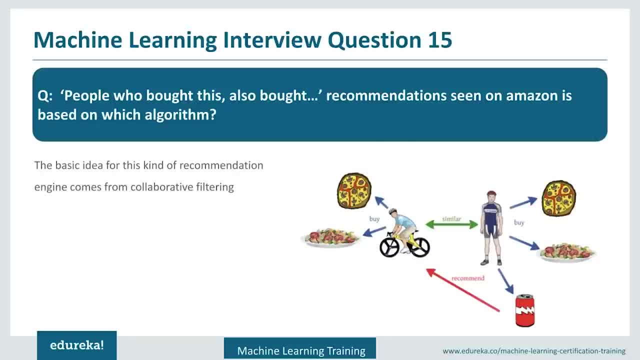 so that is the content base recommendation. what we are seeing currently for this example, it is collaborative filtering. in collaborate refiltering, what happens is what you are doing or whatever you have done previously. based on that, you will be checked with the other users who have done similar activity and it will also check what are all different activities they have. 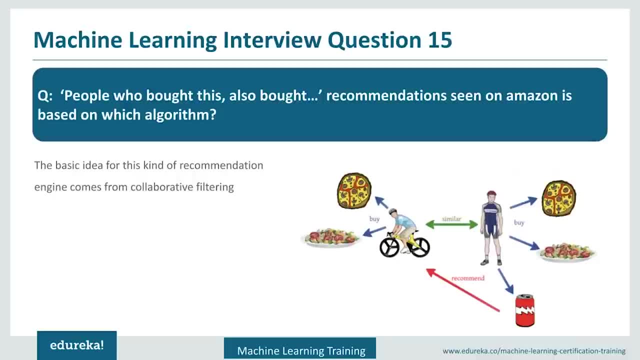 done and you have not done that, it will try to recommend those things to you. so if we see the example which is here, it says that the user who's on bicycle has brought pizza and pasta. similarly, he is trying to be compared with the user who has done similar activity. 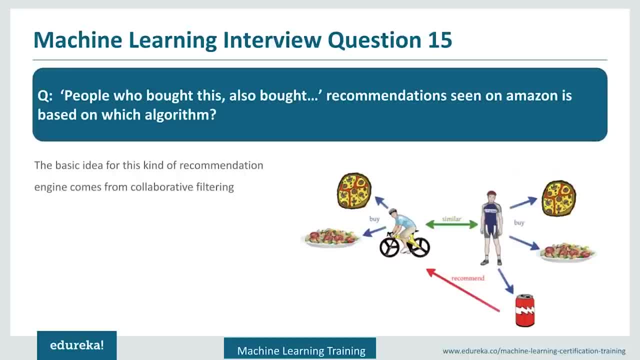 so in our case, there is this user who has brought pizza, pasta plus a coke. so as the user has not brought coke, he will be recommended this coke. so this is the core of collaboratory filtering. so this is the technique which all the major e-commerce related companies use to recommend. 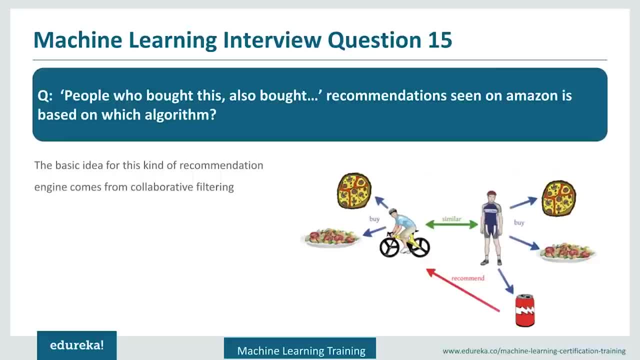 products to the users. so even netflix is just uses the content-based filtering for recommending the products based on the history that he have done, but also he'll be recommended based on the collaborative filtering, as what all other users have done similarly and what they have done as. 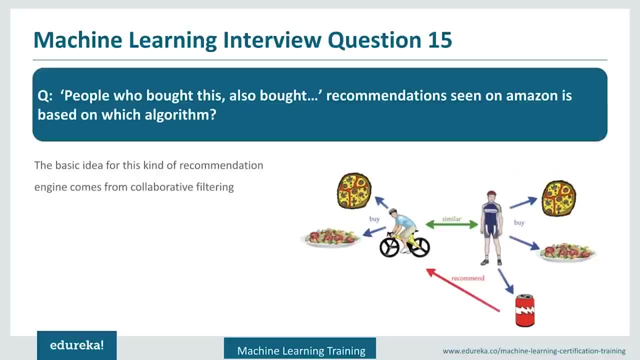 additional things. so that's how the recommendation systems works, just to summarize what we have done today. so basically we have started with the three components, three types of interview questions. we started with the core machine learning components, which involved more of a theoretical components in the machine learning. the second was we looked into. 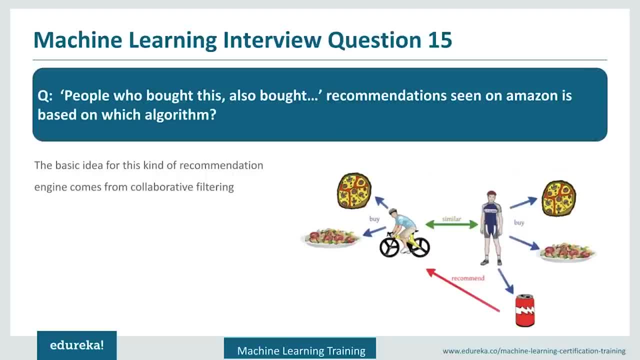 the python related questions on machine learning, we saw some practical aspects: what are the different components within python, how we can write some python code, how interviewer will try to gauge you how you can write the code and those things. and the last part was scenario based questions. so in that case we were trying to understand how, based on the scenario which is 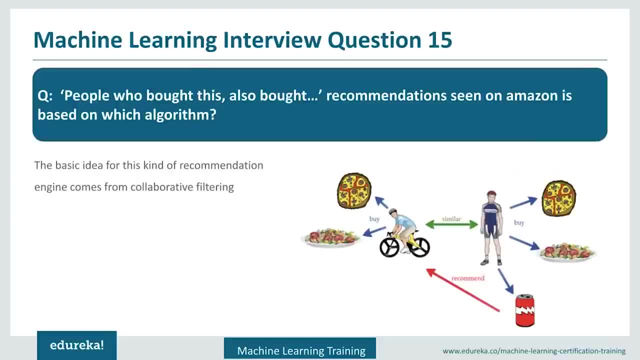 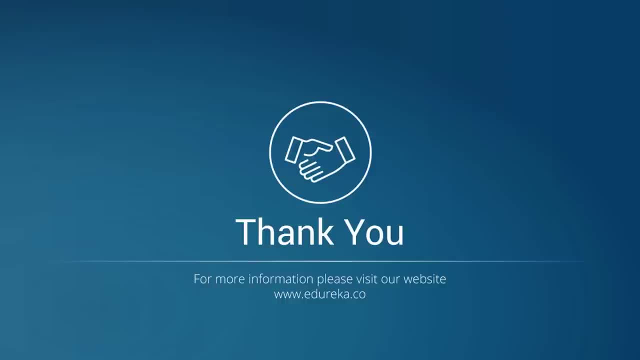 given how we can write the code and how we can write the code. and how we can write the code, how would we choose different models? how would we do the machine learning related task based on the scenario which is available to us? so i hope you all enjoyed this session and best of luck to you all.